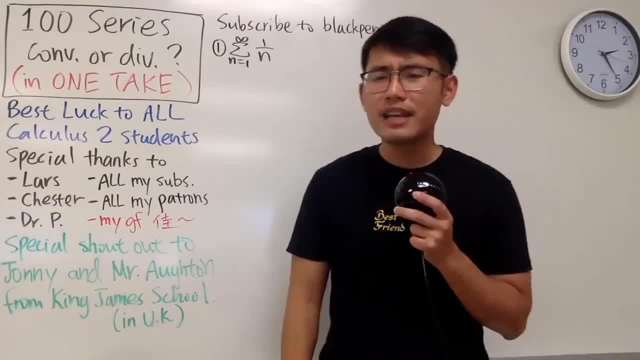 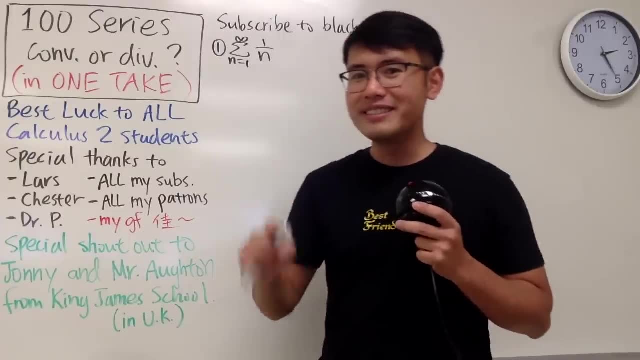 Yes, I am serious. Well, maybe today I should say that I'm serious because we'll be doing 100 series, We'll test them out if they converge or they diverge And, of course, we'll be doing this in one take. 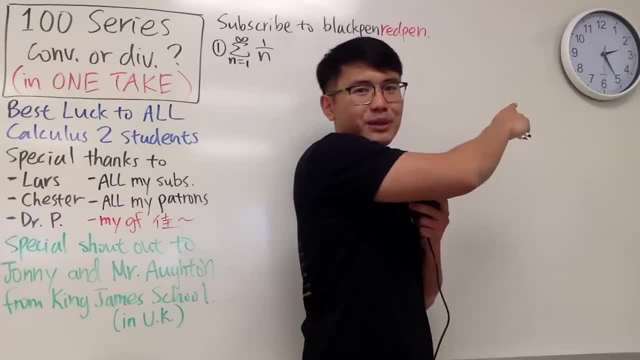 But I don't know how long this will take me. As you guys can see, that's the clock that you guys like. It's on the board already, But take a guess, how did I put the clock on the board? So leave a comment down below and let me know. 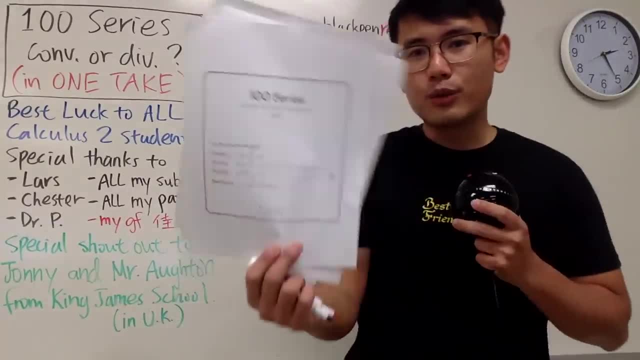 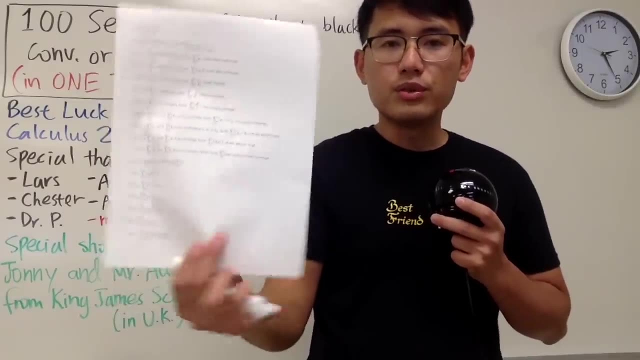 Anyway, let me tell you guys that this right here is good for Cal 2 and I have the file right here already And of course I'll be working this out along the way. You guys can go download this. The link to the PDF is in the description. 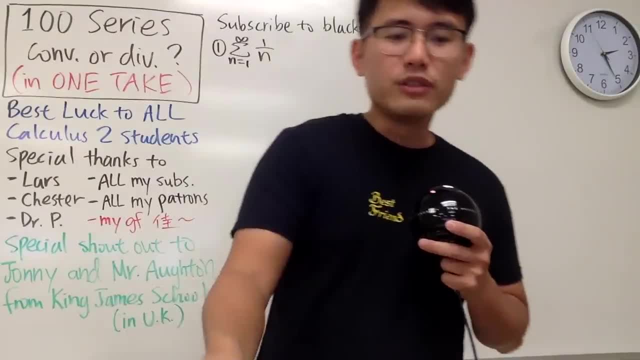 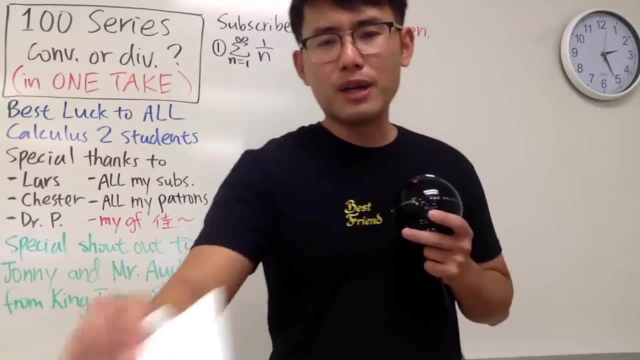 And I did spend a lot of time selecting all these questions for you guys. So please give this video a like And if you're new to my channel, hopefully you can subscribe. Thank you so much And good luck to everybody who is taking Cal 2.. 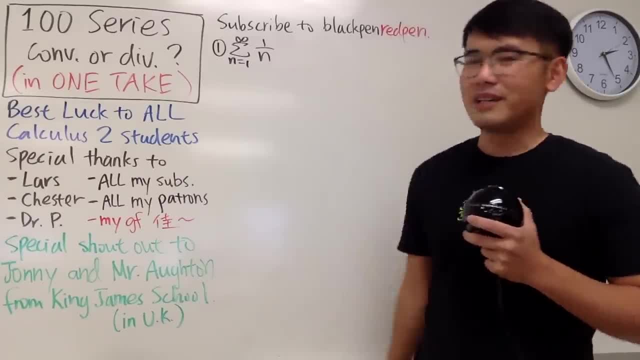 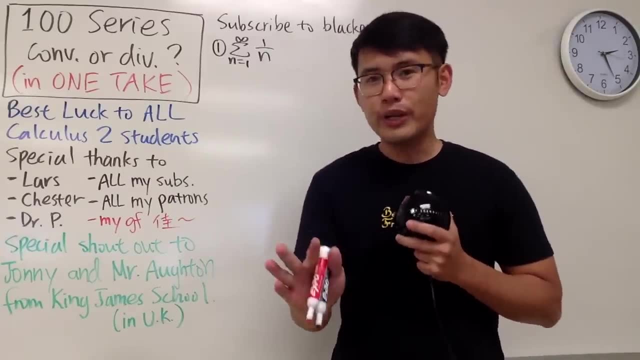 So best of luck to you guys if you have to take a Calculus 2 final exam soon. So thank you. So hopefully this will be helping you And, of course, my students. don't worry, I'm not going to give you guys 100 integrals, 100 series on the final exam. 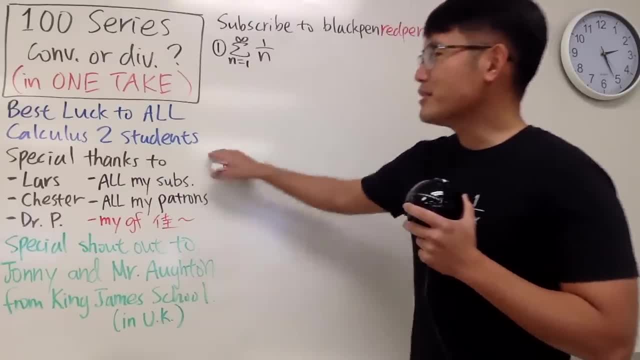 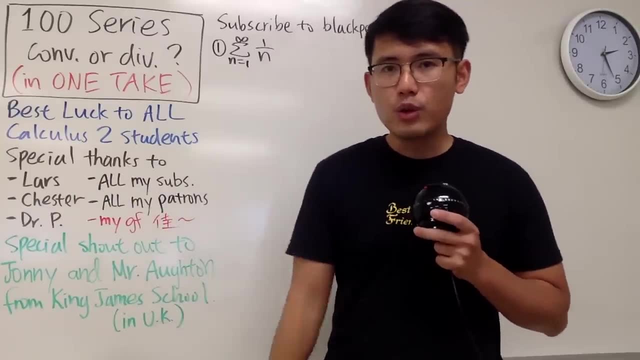 Don't worry, Just like 15.. Anyway, special thanks. I want to mention a few people before I start. First of all, Lars- And if you guys have watched my 100 integral video, you guys should know that Lars was battling, and he's still battling, with cancer. 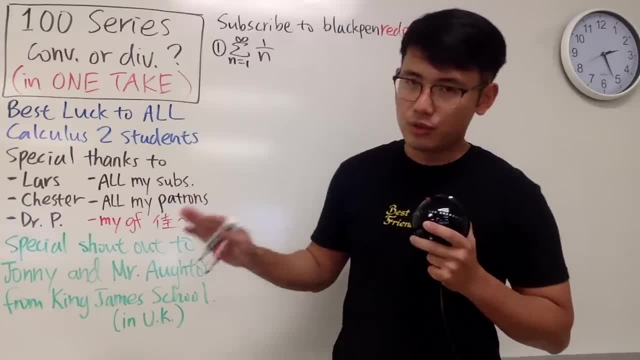 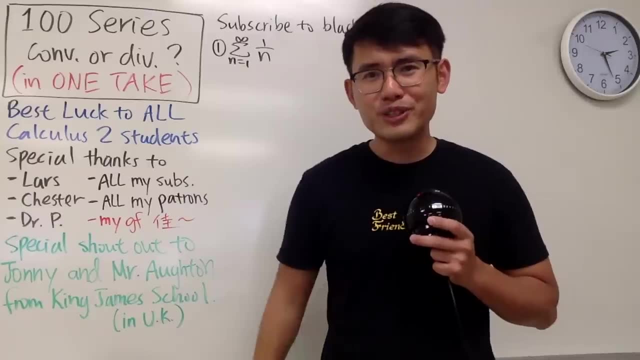 But the good news is that he's almost done with all of his treatment. So that's the good news. So he's almost cancer-free And, Lars, I want to tell you that you're an awesome person. Thank you so much for all the message. 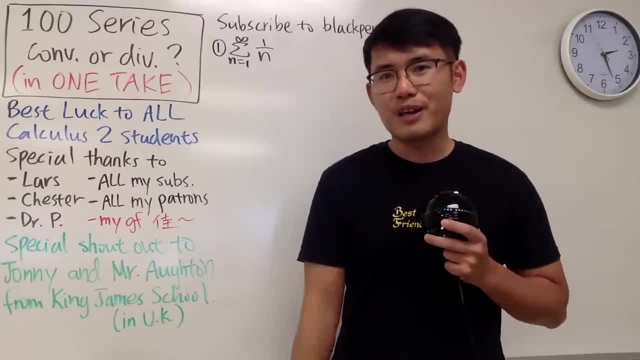 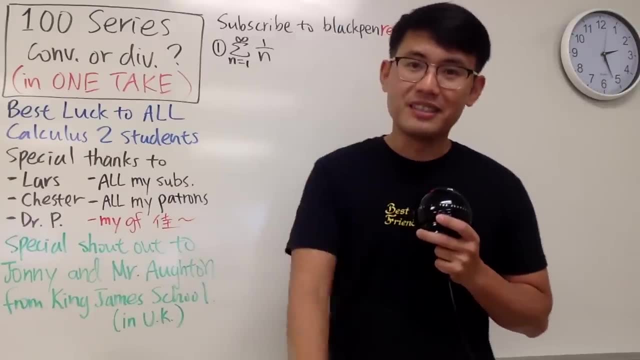 And thank you so much for the support that you have given me and Dr Payam. Yeah, you understand us, Thank you. And next I want to mention Chester. You are just as an awesome man as well, And for the other viewer, let me tell you guys that Chester is actually going to be on a military duty soon. 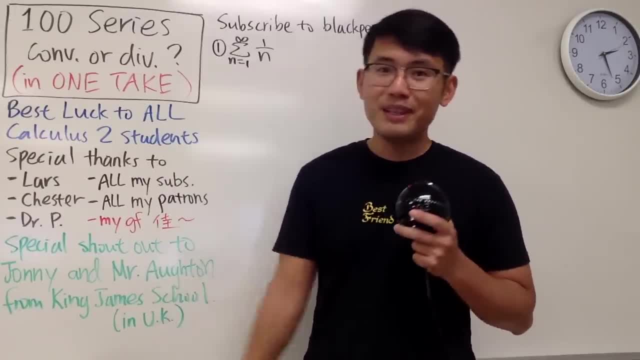 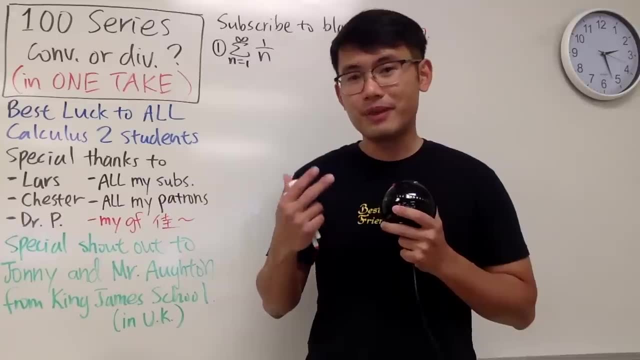 He's going to be away to another country for nine months And it's amazing. It's amazing that he is watching my video and I find it's just so amazing, Thank you. Thank you for your service And you know I really enjoy the conversation that we have about math or maybe about other things as well. 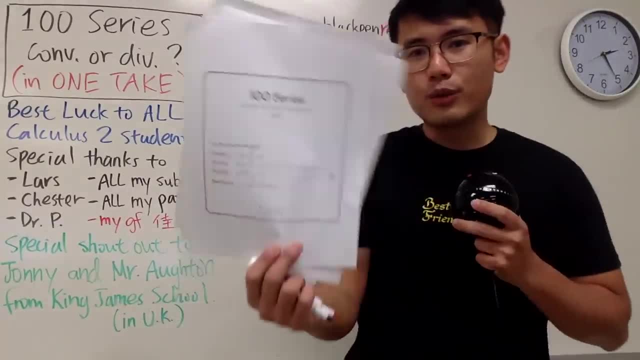 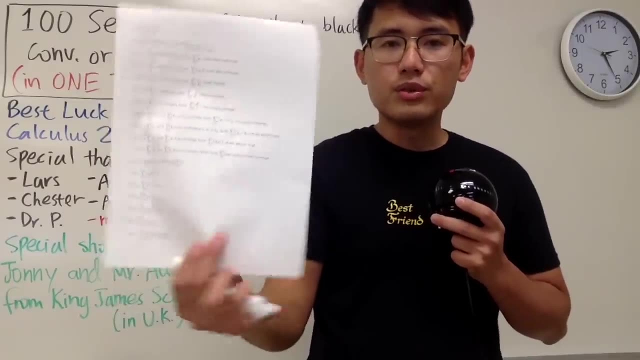 Anyway, let me tell you guys that this right here is good for Cal 2 and I have the file right here already And of course I'll be working this out along the way. You guys can go download this. The link to the PDF is in the description. 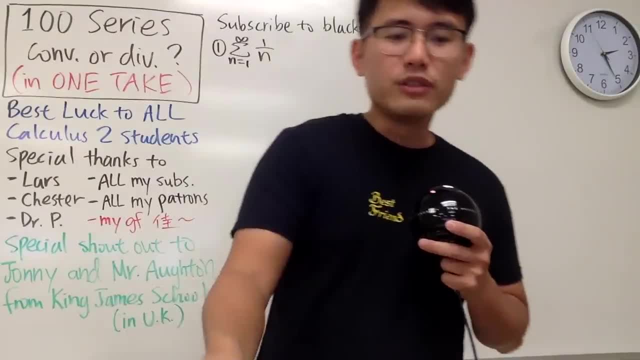 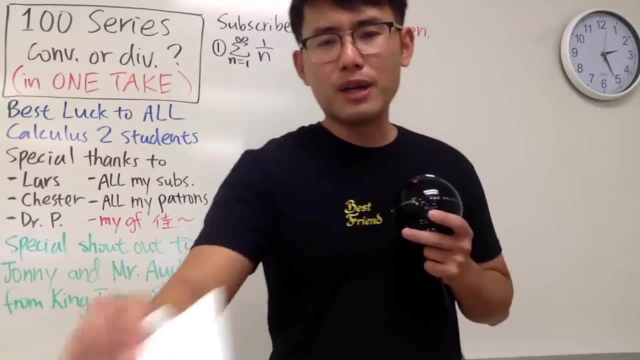 And I did spend a lot of time selecting all these questions for you guys. So please give this video a like And if you're new to my channel, hopefully you can subscribe. Thank you so much And good luck to everybody who is taking Cal 2.. 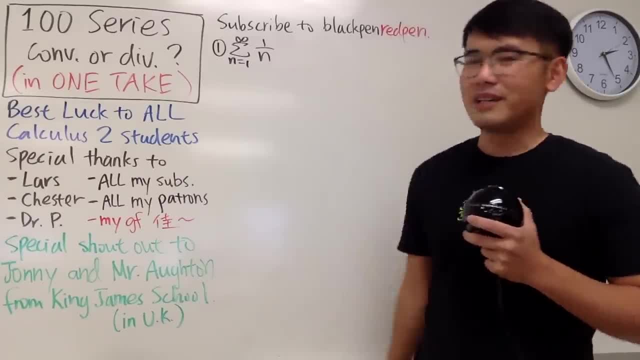 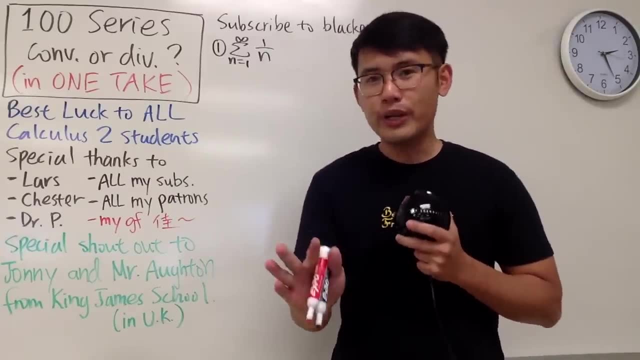 So best of luck to you guys if you have to take a Calculus 2 final exam soon. So thank you. So hopefully this will be helping you And, of course, my students. don't worry, I'm not going to give you guys 100 integrals, 100 series on the final exam. 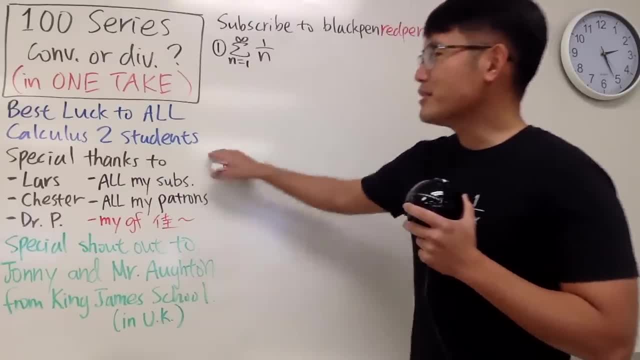 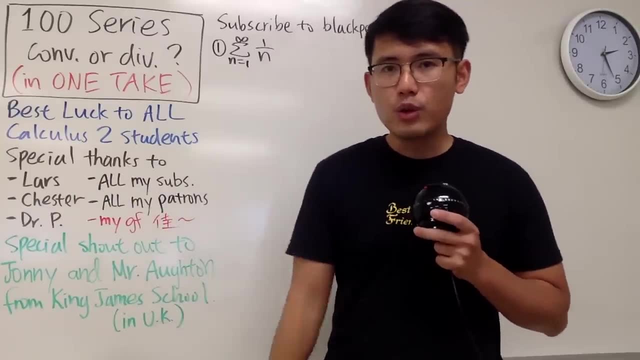 Don't worry, Just like 15.. Anyway, special thanks. I want to mention a few people before I start. First of all, Lars- And if you guys have watched my 100 integral video, you guys should know that Lars was battling, and he's still battling, with cancer. 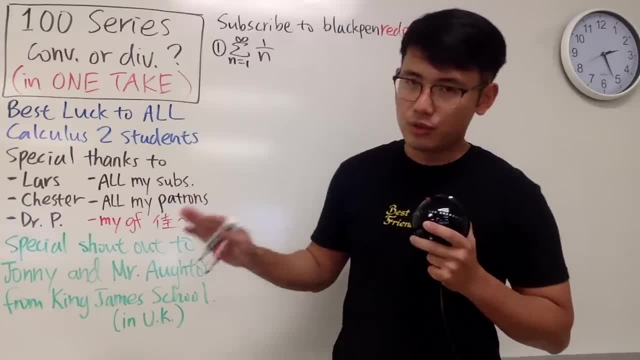 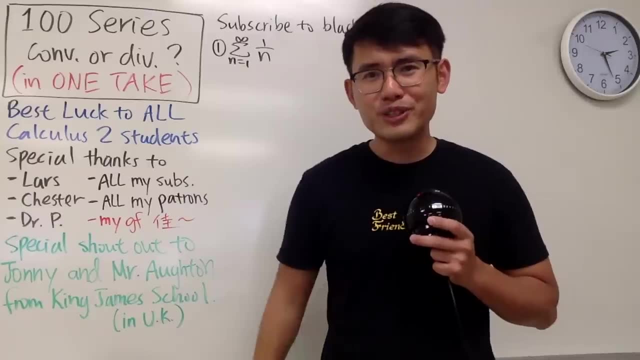 But the good news is that he's almost done with all of his treatment. So that's the good news. So he's almost cancer-free And, Lars, I want to tell you that you're an awesome person. Thank you so much for all the message. 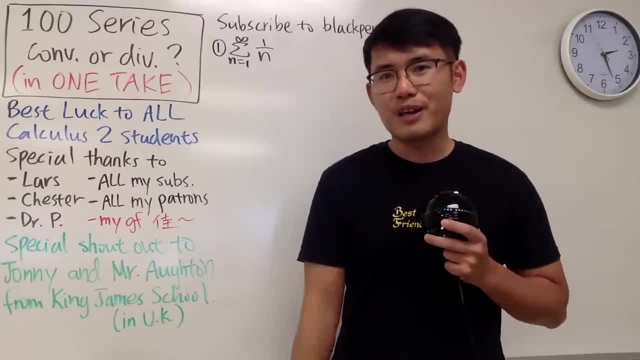 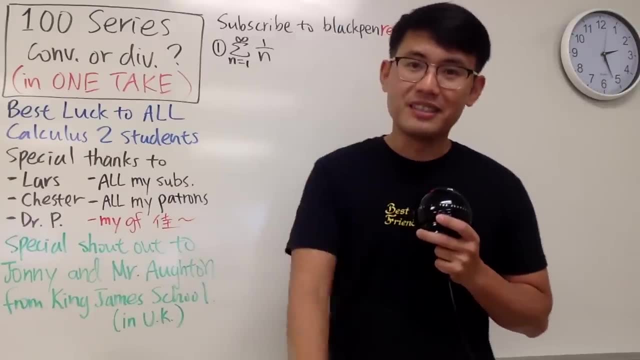 And thank you so much for the support that you have given me and Dr Payam. Yeah, you understand us, Thank you. And next I want to mention Chester. You are just as an awesome man as well, And for the other viewer, let me tell you guys that Chester is actually going to be on a military duty soon. 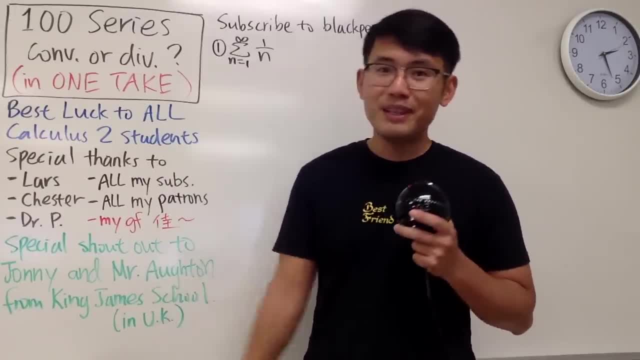 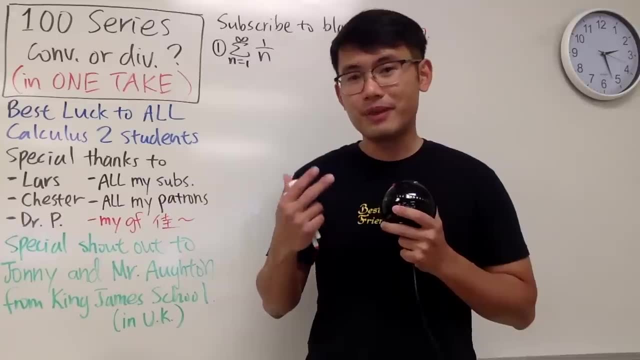 He's going to be away to another country for nine months And it's amazing. It's amazing that he is watching my video and I find it's just so amazing, Thank you. Thank you for your service And you know I really enjoy the conversation that we have about math or maybe about other things as well. 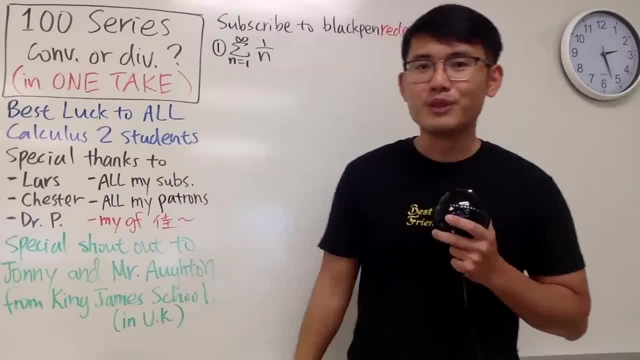 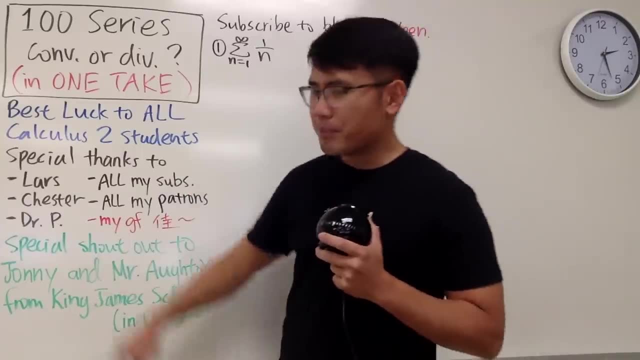 And I want to wish you the best of luck. Again, thank you for your service And, you know, hopefully we get to meet each other in SoCal one day soon. Next, of course, Dr P. If you guys don't know who Dr P is, of course check the link in the description. 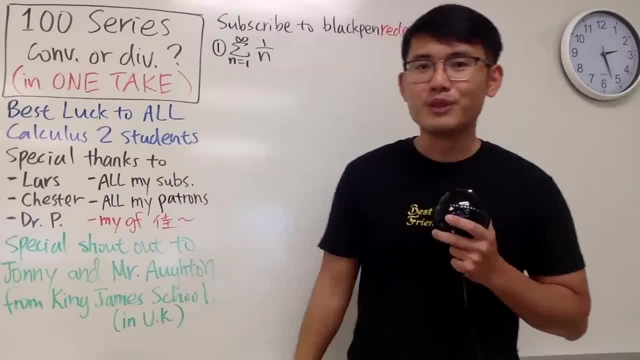 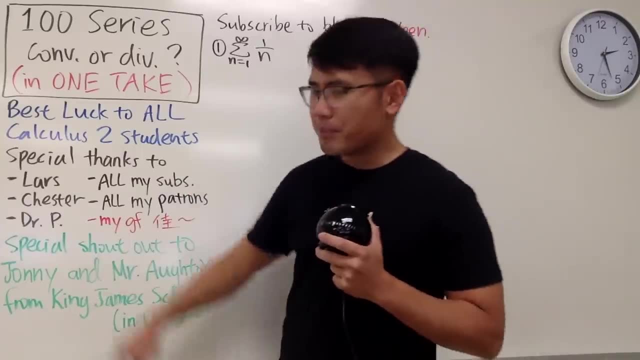 And I want to wish you the best of luck. Again, thank you for your service And, you know, hopefully we get to meet each other in SoCal one day soon. Next, of course, Dr P. If you guys don't know who Dr P is, of course check the link in the description. 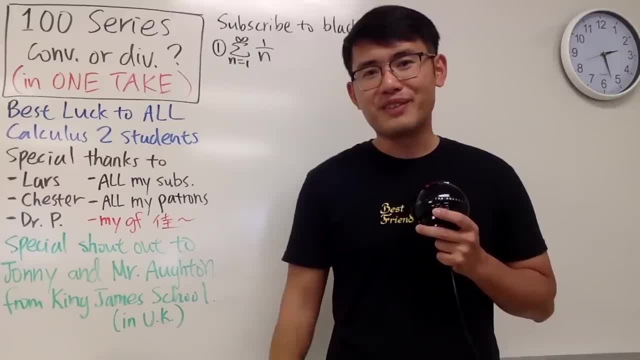 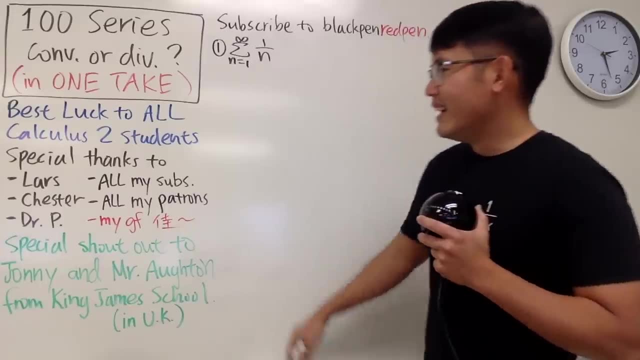 You will see that he is the happiest mathematician ever, Right, Good friend of mine, If you are watching Dr P, just leave a comment down below too, And of course I will have to say that you know. 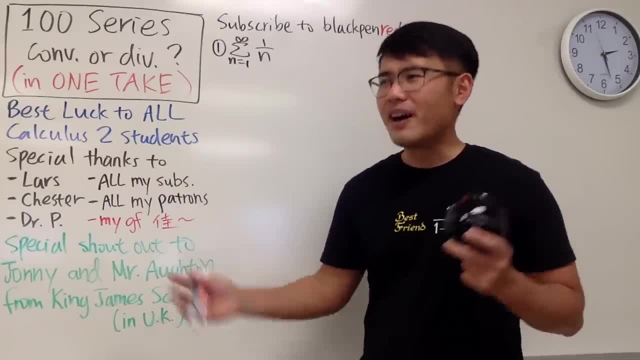 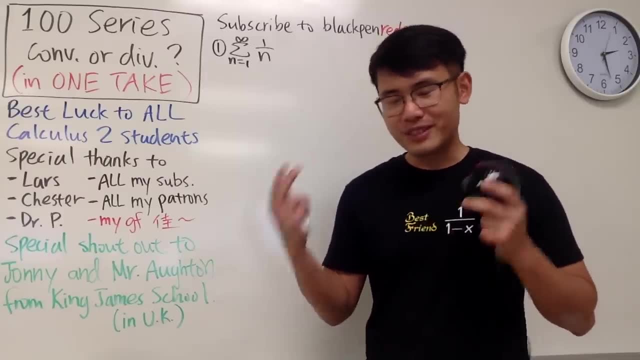 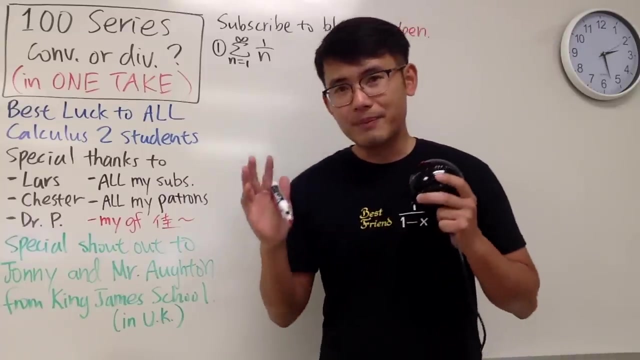 without you guys. seriously, where is the fun of doing videos without all my subscribers? It's amazing And I just want to say thank you To all my subscribers, all my supporters, all my Patreons. you guys are so amazing. You guys are seriously. 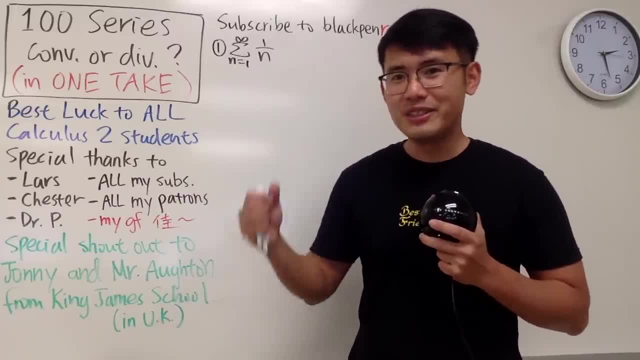 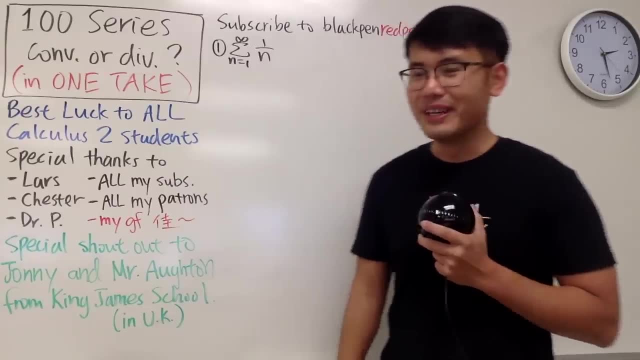 the reasons why I still have the energy, the motivation, the motivation to keep this channel going And, of course, I will continue to do so for you guys, Thank you, And my girlfriend Jia. You know I love my girlfriend. 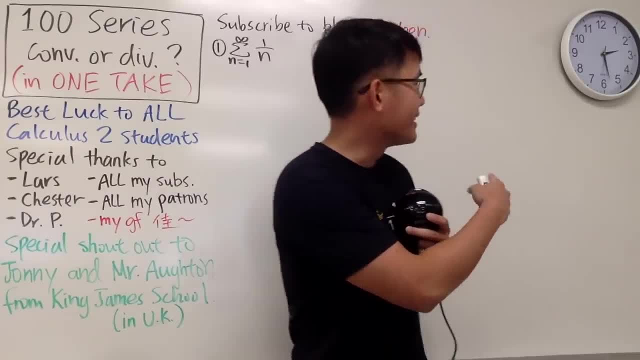 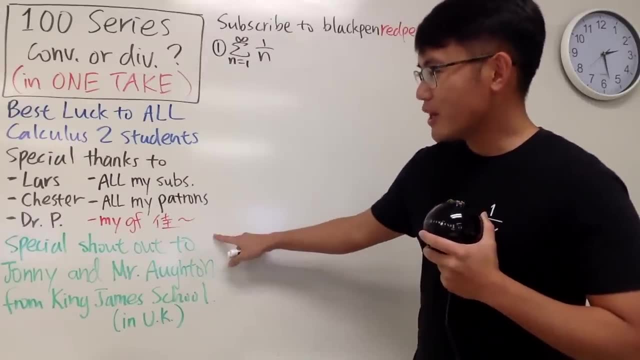 I don't know how long this will take me. Hopefully I will finish within like six hours maybe, But I don't know. But after this video I will go see you, Of course. Special shout-out to Johnny and Mr Alton. 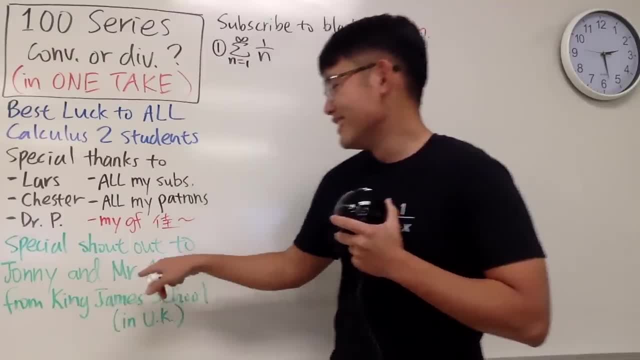 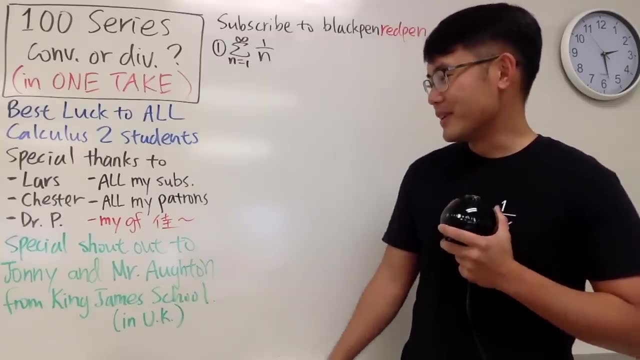 All the way from UK King James School. I think this right here has nothing to do with Le Bon James, but like, if it does, let me know. right, But it's a school in the United Kingdom, But yeah, Anyway. 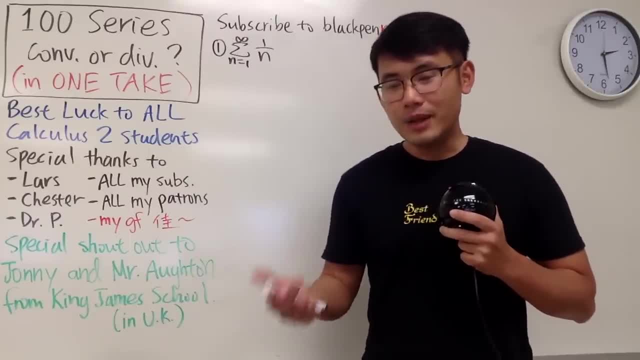 thank you for your message, Johnny, And thank you for your support. I actually made a video to give you guys a shout-out, but like I wasn't satisfied with the math, that I did in that video, So you know. 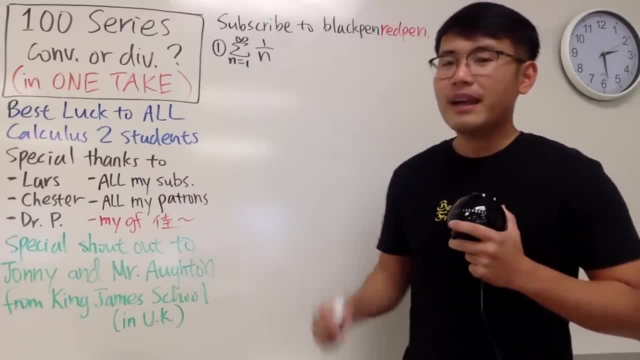 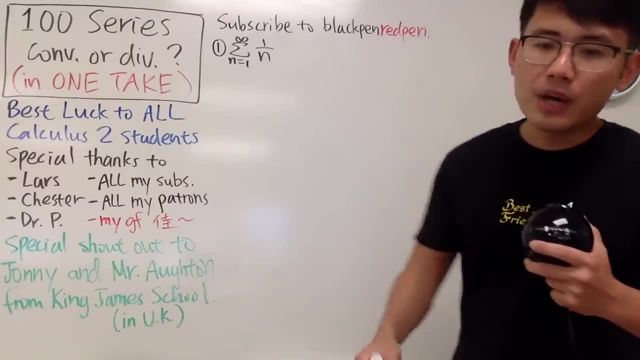 I put that unlisted. Now, this is for you guys. And lastly, of course, please subscribe to BlackPinkRedPen. Thank you guys so much. You guys are awesome. Alright, so here we go. First of all, you guys should look at the cover page. 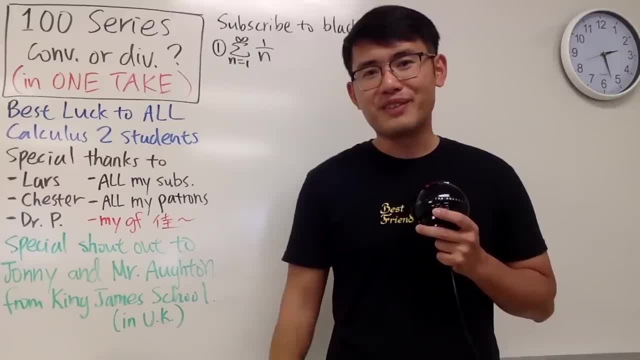 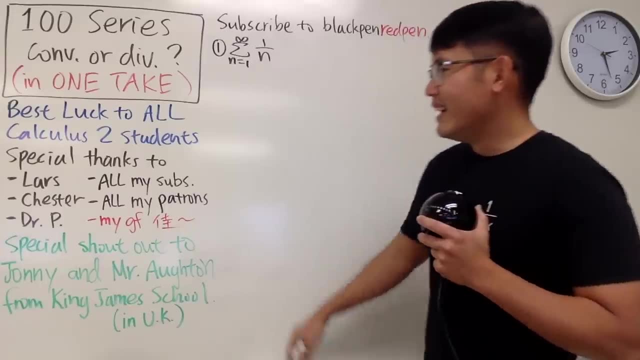 You will see that he is the happiest mathematician ever, Right, Good friend of mine, If you are watching Dr P, just leave a comment down below too, And of course I will have to say that you know. 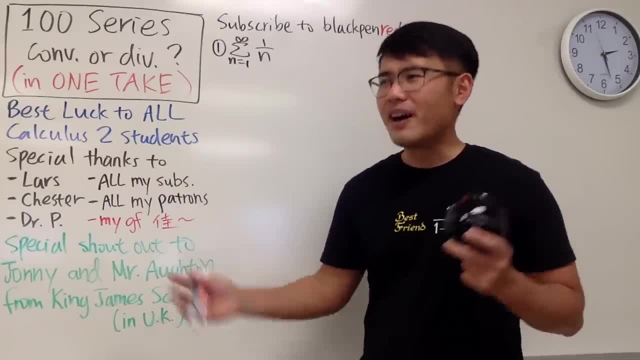 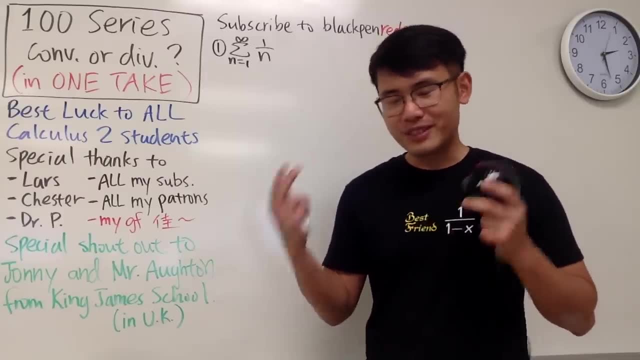 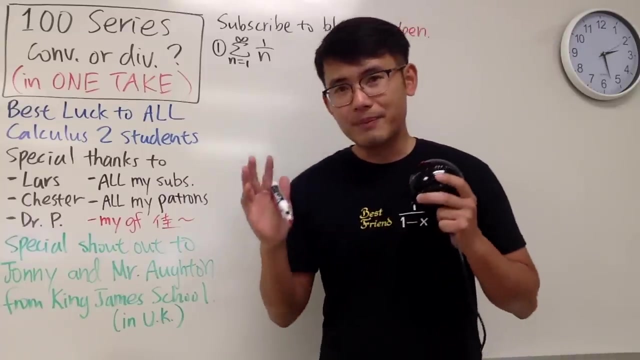 without you guys. seriously, where is the fun of doing videos without all my subscribers? It's amazing And I just want to say thank you To all my subscribers, all my supporters, all my Patreons. you guys are so amazing. You guys are seriously. 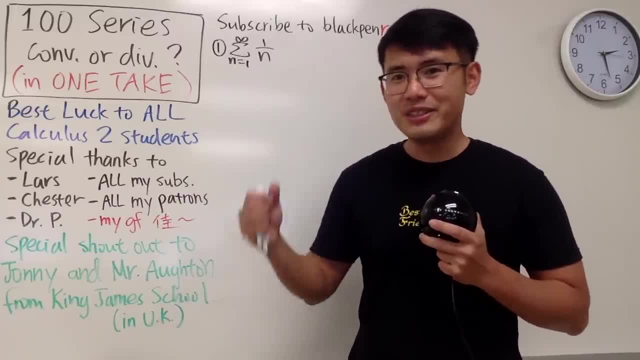 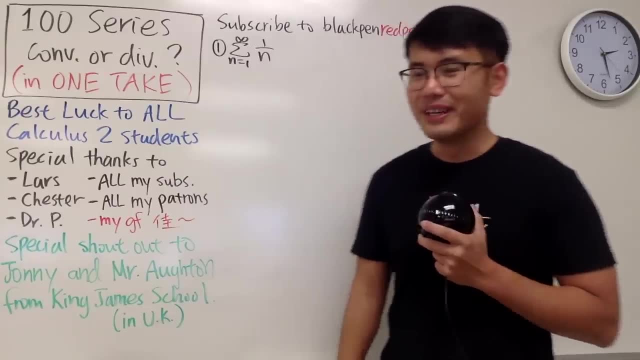 the reasons why I still have the energy, the motivation, the motivation to keep this channel going And, of course, I will continue to do so for you guys, Thank you, And my girlfriend Jia. You know I love my girlfriend. 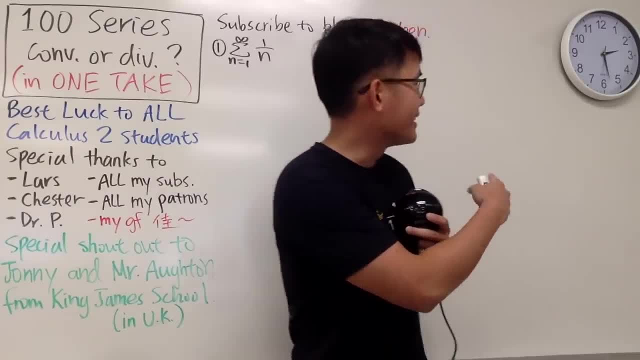 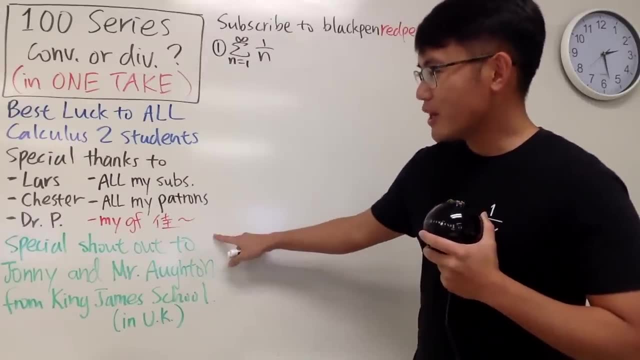 I don't know how long this will take me. Hopefully I will finish within like six hours maybe, But I don't know. But after this video I will go see you, Of course. Special shout-out to Johnny and Mr Alton. 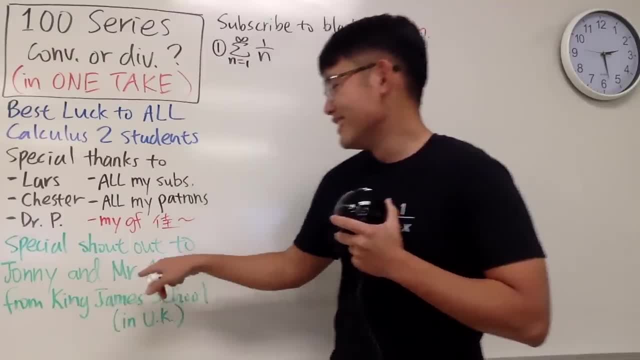 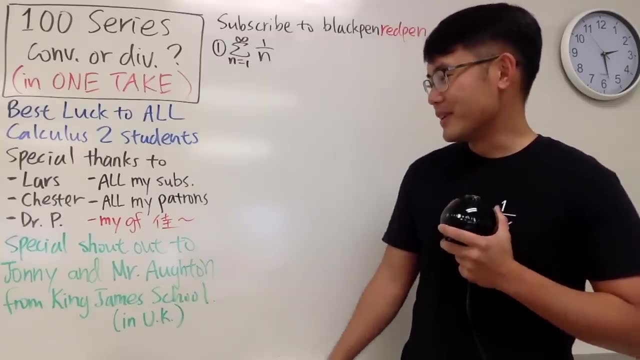 All the way from UK King James School. I think this right here has nothing to do with Le Bon James, but like, if it does, let me know. right, But it's a school in the United Kingdom. But yeah, Anyway, thank you. 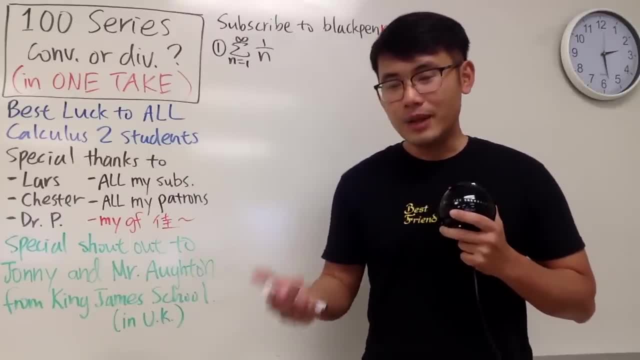 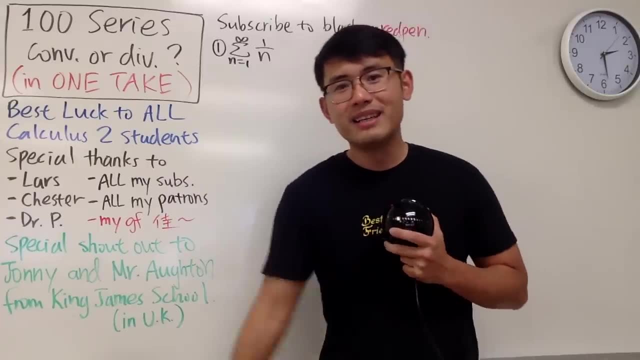 for your message, Johnny, And thank you for your support. I actually made a video to give you guys a shout-out, but like I wasn't satisfied with the math, that I did in that video, So you know I put that and list it. Now this is it. 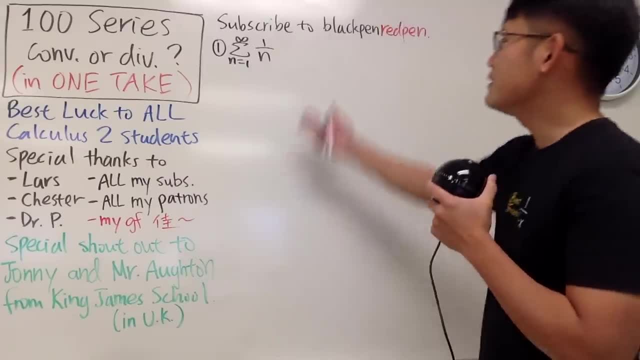 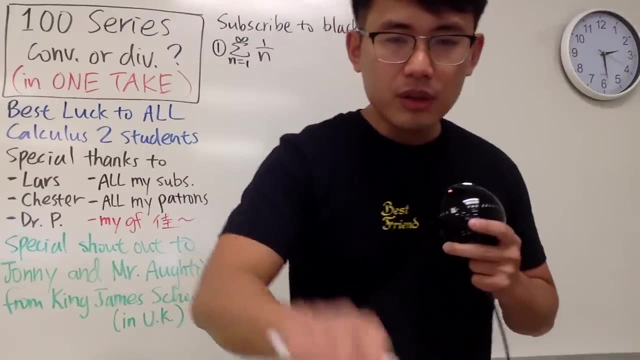 This is for you guys. And lastly, of course, please subscribe to BlackPenRedPen. Thank you guys so much. You guys are awesome. Alright, so here we go. First of all, you guys should look at the cover page. 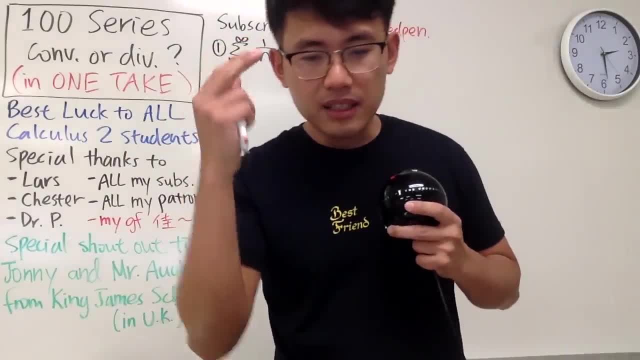 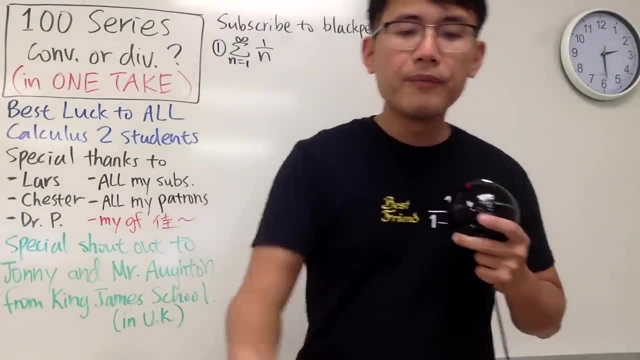 I have the four secret weapons, Namely the fact, the list, the limit and also the best friend. So be sure you know all that. I will be just referring to these things right here along the way. And here we go. First question: 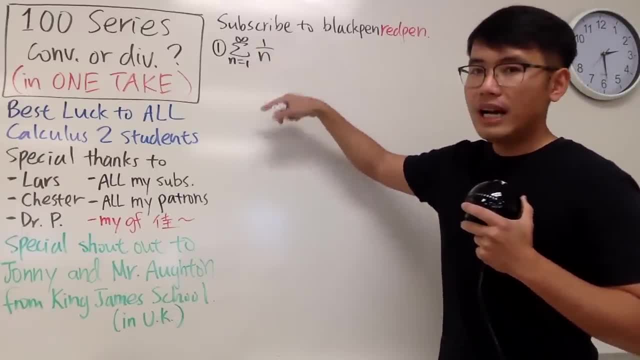 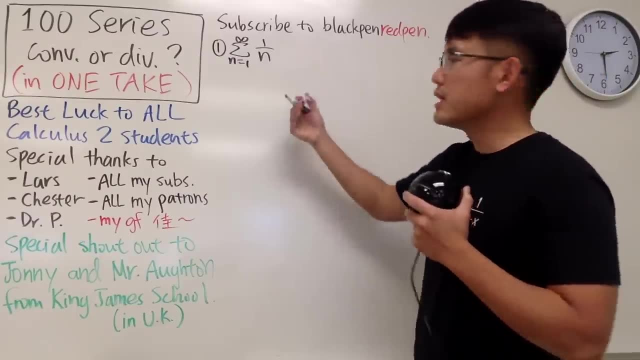 We have the sum, as n goes from 1 to infinity, of 1 over n to the first power And, as you all know, this right here diverges. right, because you can see that this is the p-series. Well, you can say: 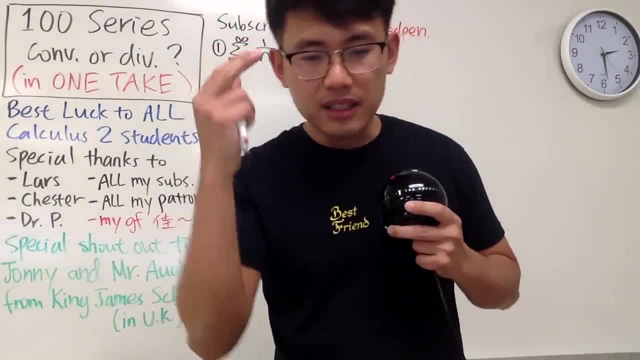 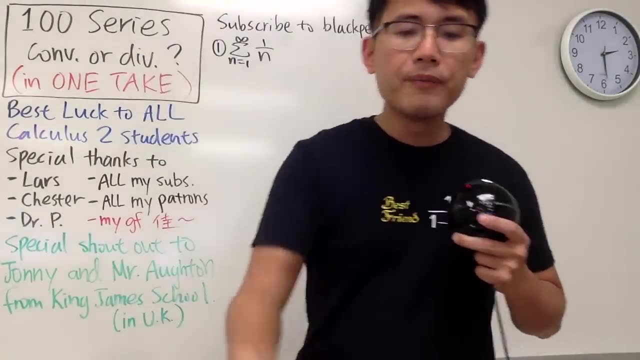 I have the four secret weapons, Namely the fact, the list, the limit and also the best friend. So be sure you know all that. I will be just referring to these things right here along the way. And here we go. 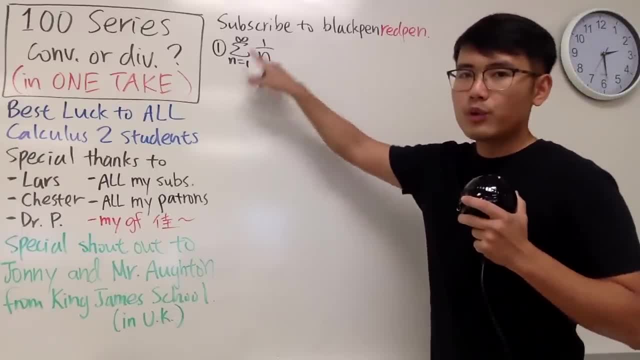 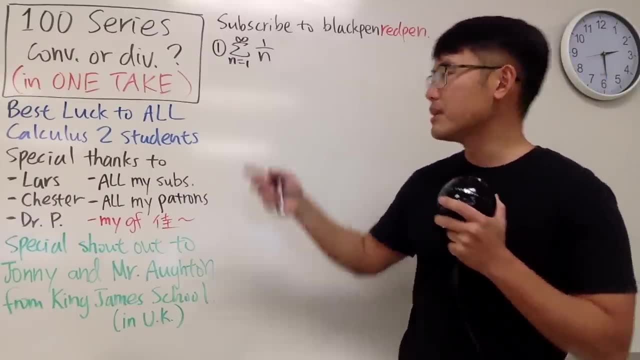 First question: We have the sum, as n goes from 1 to infinity, of 1 over n to the first power And, as you all know, this right here diverges. Right, Because you can see that this is the p-series. Well, you can say: 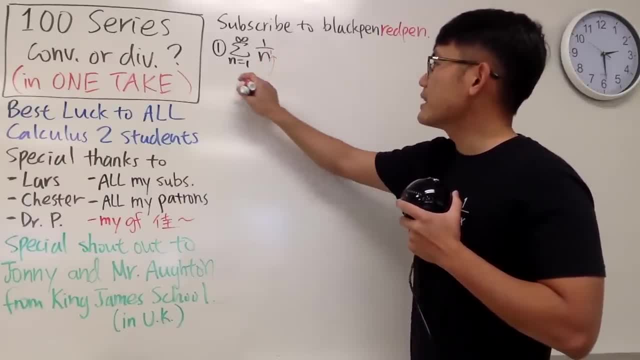 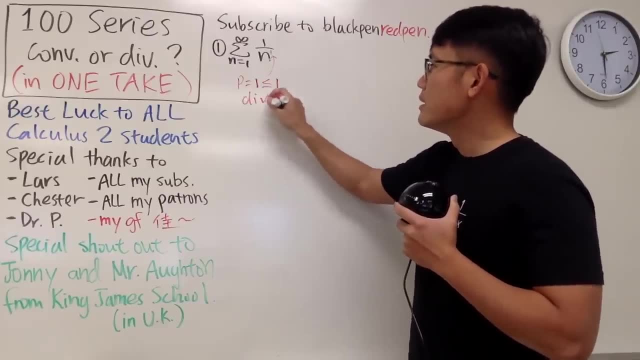 that's n to the first power. and when you do that, you can indicate that p is equal to 1, which is less than or equal to 1.. Right, That's important right here. And this right here diverges. 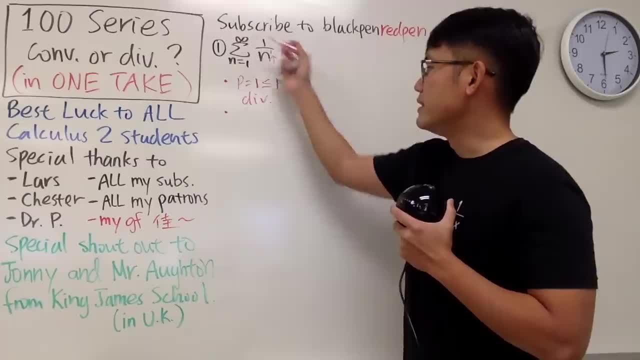 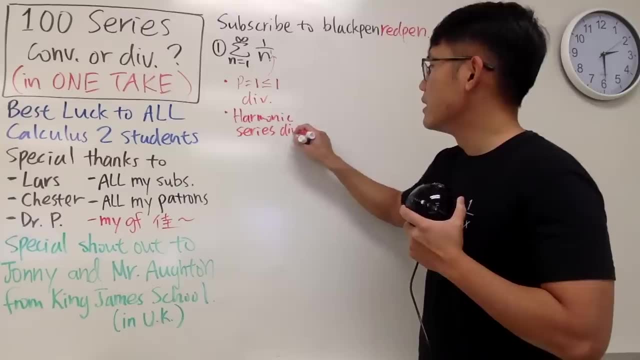 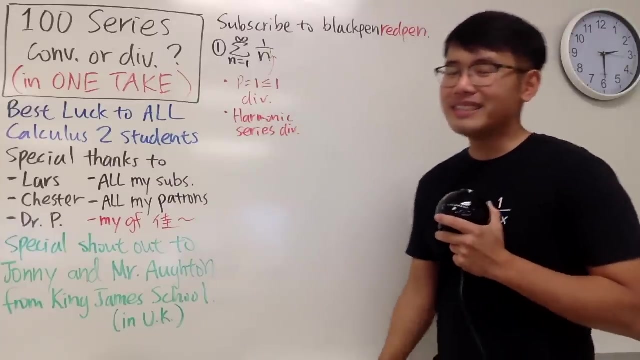 Or you can also say that this right here is the famous harmonic series, and you can just say that harmonic series diverges. That's fine too, But have you guys ever seen the proof of this? Well, I think this is so classic, so I'm going to do this one right here. 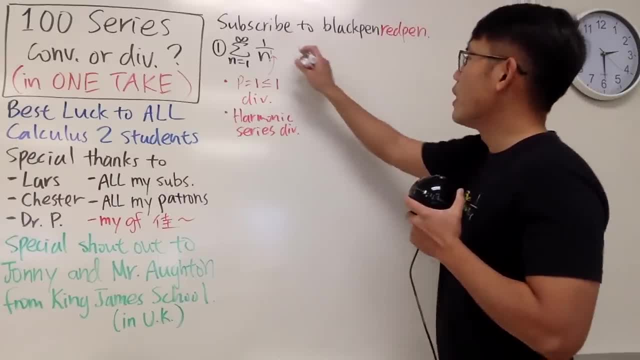 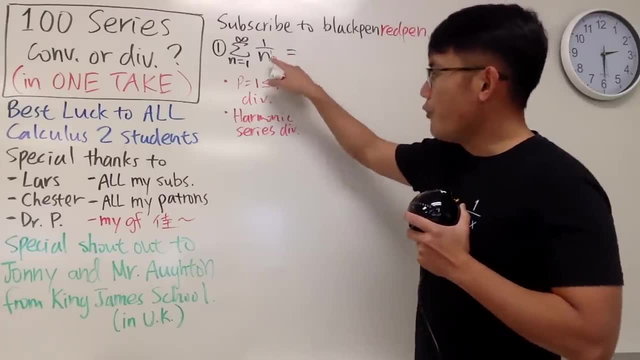 for you guys as the first question. So here we go. Let me show you guys that Look at 1 over n. The interesting part of this is that 1 over n does approach to infinity, but this right here actually diverges. 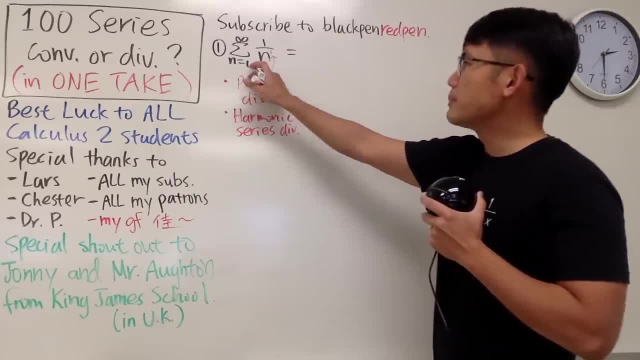 And this is the reason why. So let me show you. Let me just put the 1,, 2,, 3,, 4,, 5, and so on into the 1 over n, And we get 1 over 1. 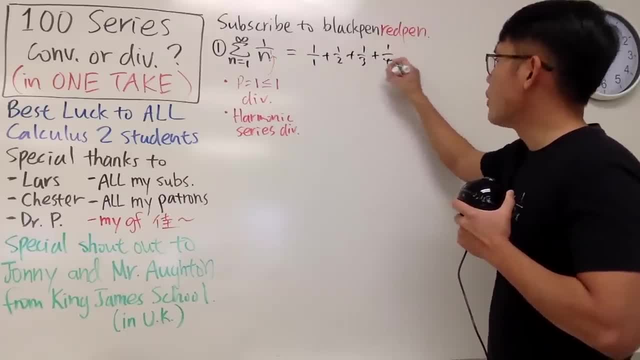 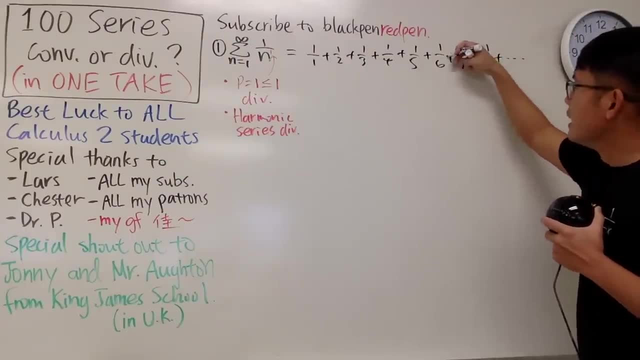 plus 1 over 2 plus 1 over 3, plus 1 over 4, plus 1 over 5, plus 1 over 6, plus 1 over 7, plus 1 over 8, plus dot dot dot, And if you want to put on more terms, 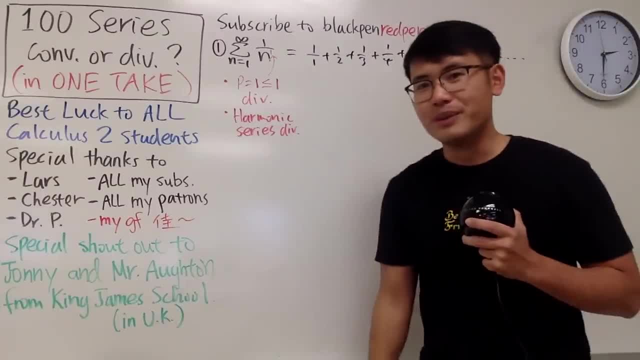 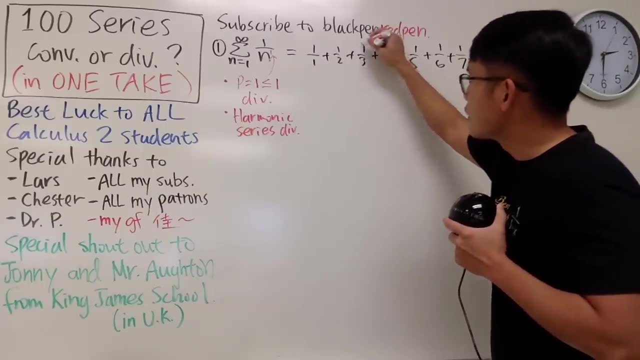 you will have to stop at 1 over 16, the powers of 2.. And this is the reason why. Okay, first of all, 1, 1 half, they are good. But for the 1 third, right here, 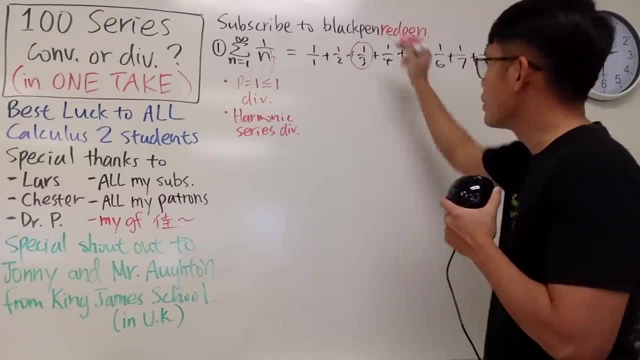 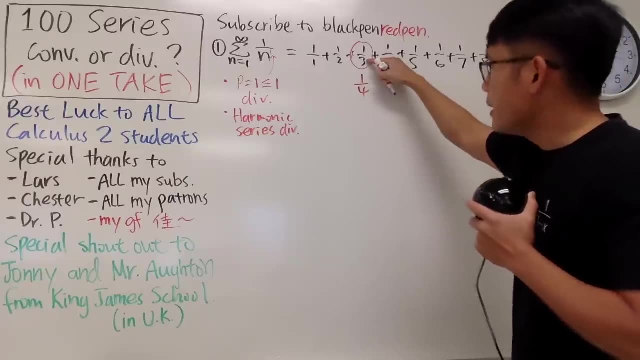 I will change that to 1 over 4.. And the connection between 1 third and 1 over 4 is that this right here is bigger than this. Check this out: If the denominator is smaller than the denominator here, while the numerators are the same. 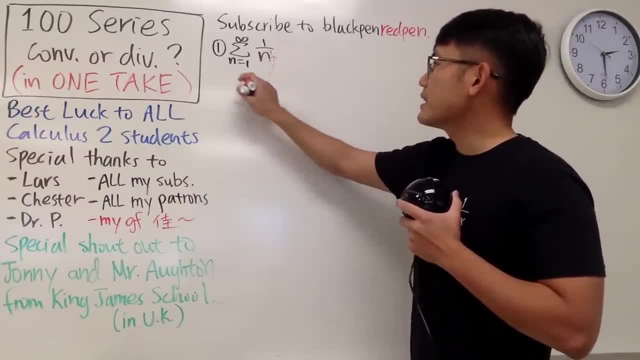 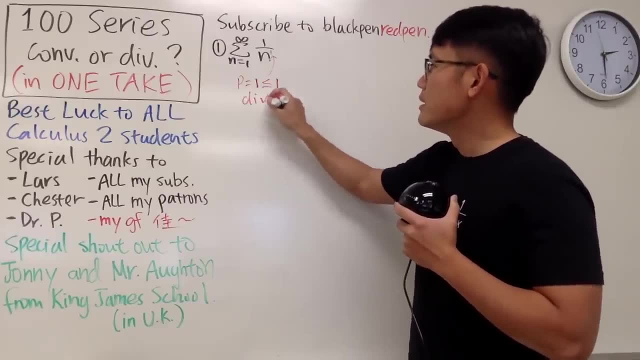 that's n to the first power. And when you do that, you can indicate that p is equal to 1, which is less than or equal to 1.. Right, that's important right here. And this right here diverges. Or you can also say that: 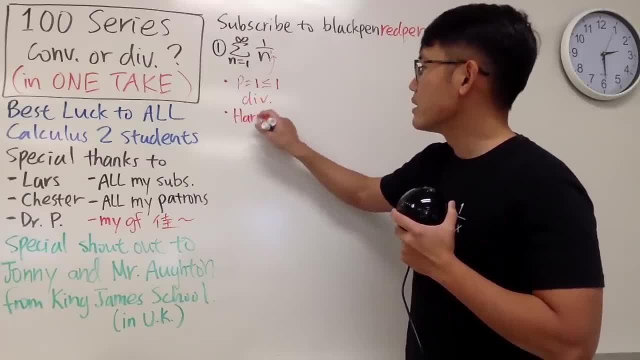 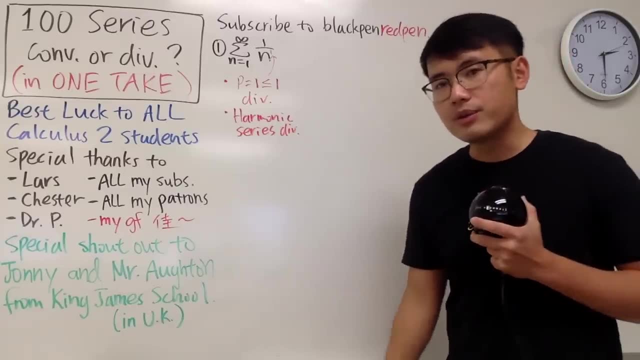 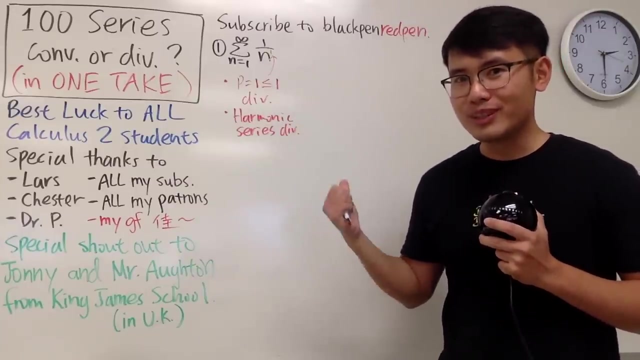 this right here is the famous harmonic series, And you can just say that harmonic series diverges. That's fine too, But have you guys ever seen the proof of this? Well, I think this is so classic, so I'm going to do this one right here. 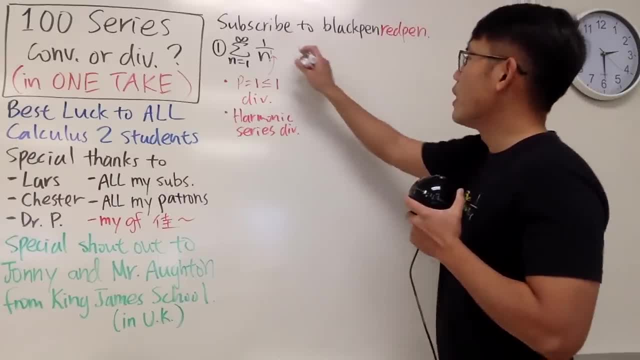 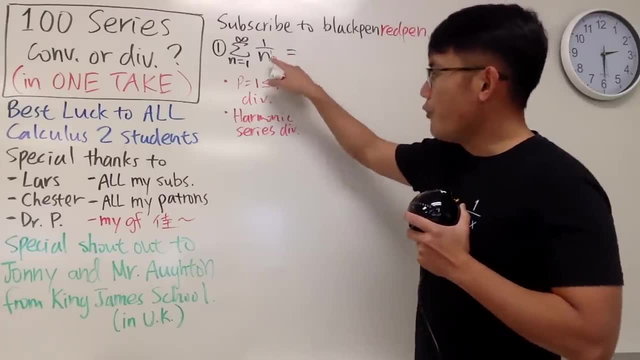 for you guys as the first question. So here we go. Let me show you guys that Look at 1 over n. The interesting part of this is that 1 over n does approach to infinity, but this right here actually diverges. 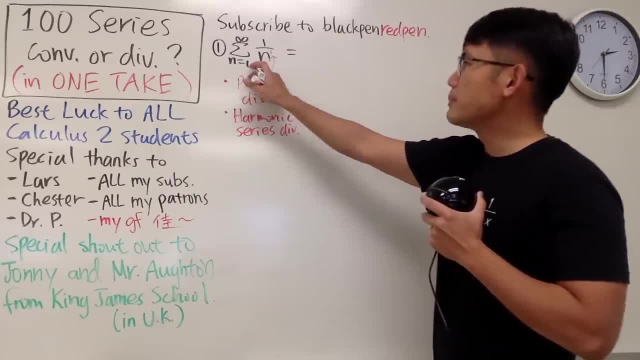 And this is the reason why. So let me show you. Let me just put the 1,, 2,, 3,, 4,, 5, and so on into the 1 over n, And we get 1 over 1. 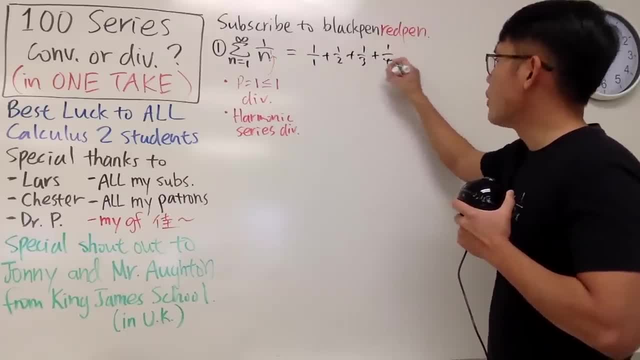 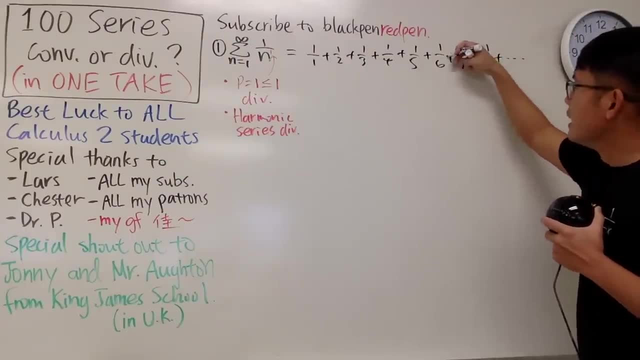 plus 1 over 2 plus 1 over 3, plus 1 over 4, plus 1 over 5, plus 1 over 6, plus 1 over 7, plus 1 over 8, plus dot dot dot, And if you want to put on more terms, 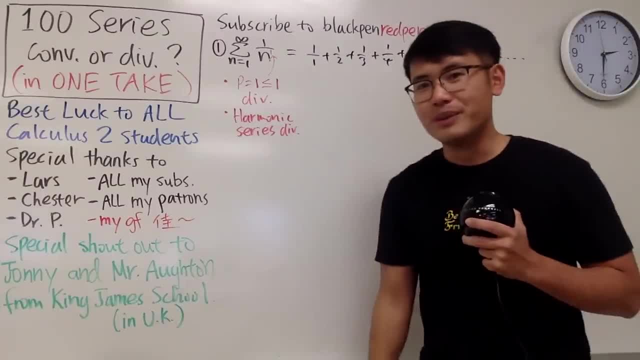 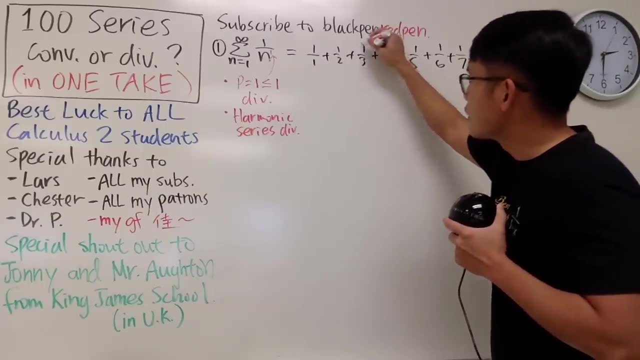 you will have to stop at 1 over 16, the powers of 2.. And this is the reason why. Okay, first of all, 1, 1 half, they are good. But for the 1 third, right here, 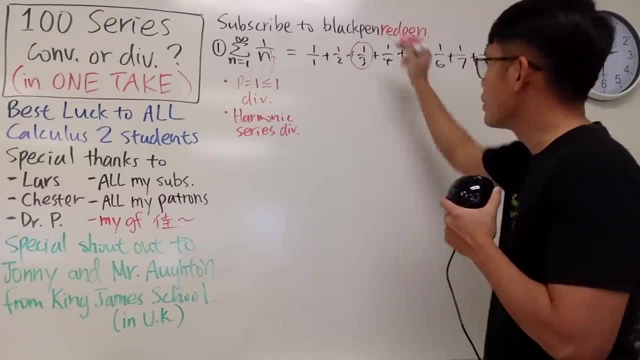 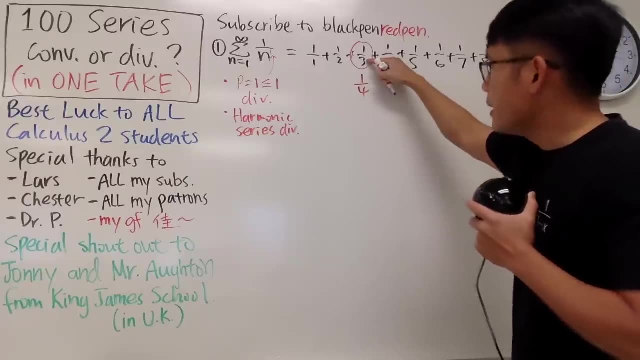 I will change that to 1 over 4.. And the connection between 1 third and 1 over 4 is that this right here is bigger than this. Check this out: If the denominator is smaller than the denominator here, while the numerators are the same. 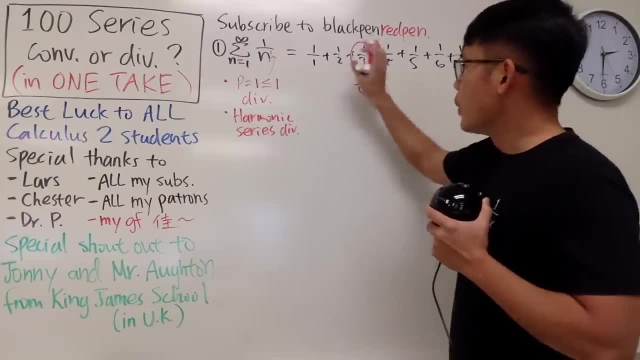 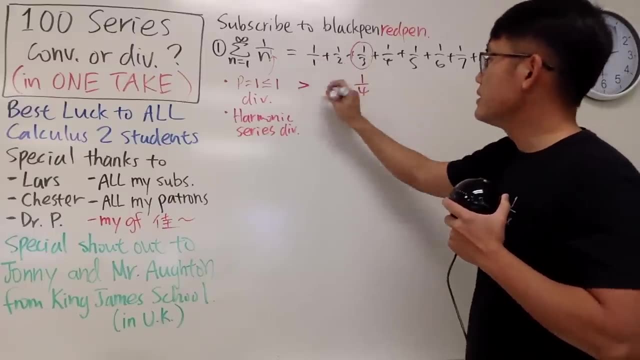 then this right here will be bigger than that Right. So when we have that, we can just put this down as okay. we can put down this, as this is greater than the following: This is still 1, so I'll keep it. 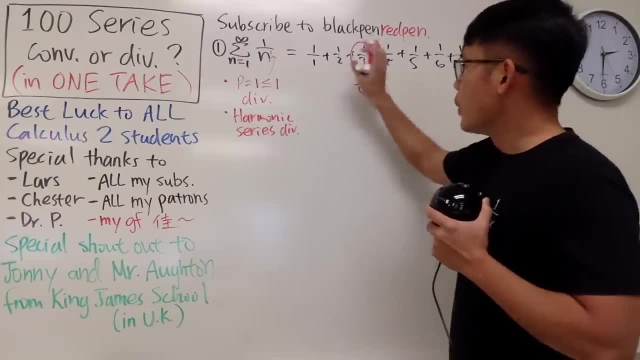 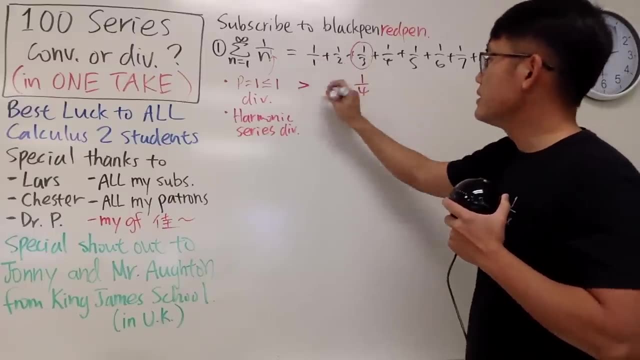 then this right here will be bigger than that Right. So when we have that, we can just put this down as okay. we can put down this as this is greater than the following: This is still 1, so keep it and then. 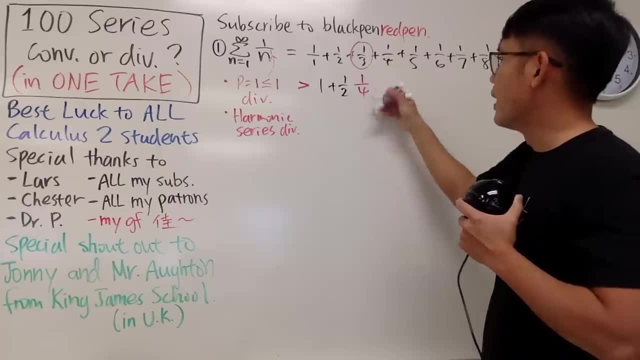 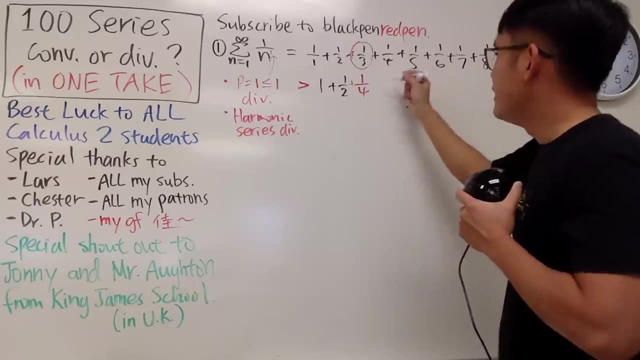 the 1 half. I will also keep that This is 1 over 4 now, but I'm saying this is greater than 1 over 4.. And of course I'll just put down plus And this 1 over 4 is still legit. 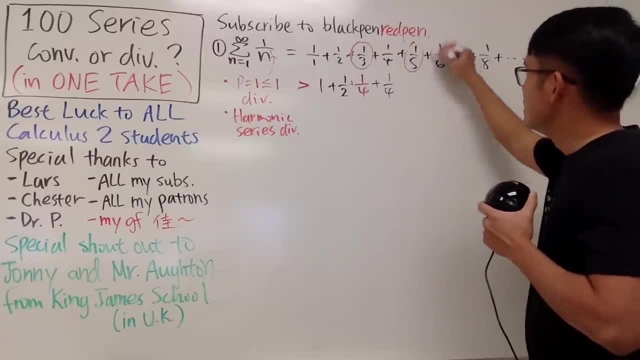 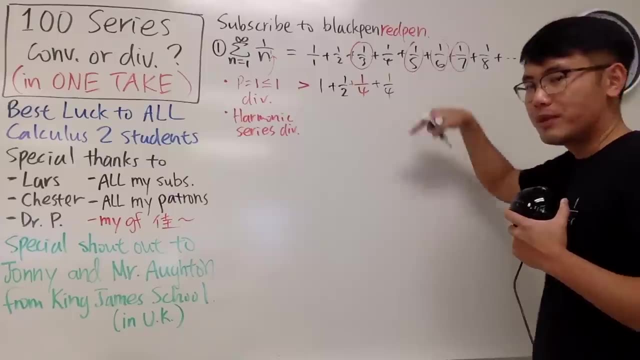 I'll just keep that down, And then for this, this and that, I will change them to 1 over 8. And of course, everybody here is bigger than 1 over 8.. So I will just put down: this is bigger than 1 over. 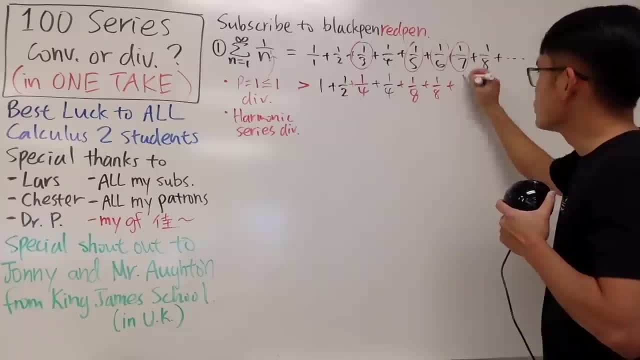 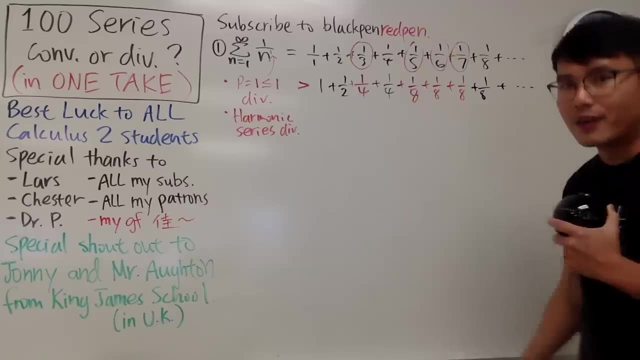 8,. this is also bigger than 1 over 8, and this is also bigger than 1 over 8, and this is the 1 over 8 itself. And then, of course, this right here keeps on going forever. Now, the beauty. 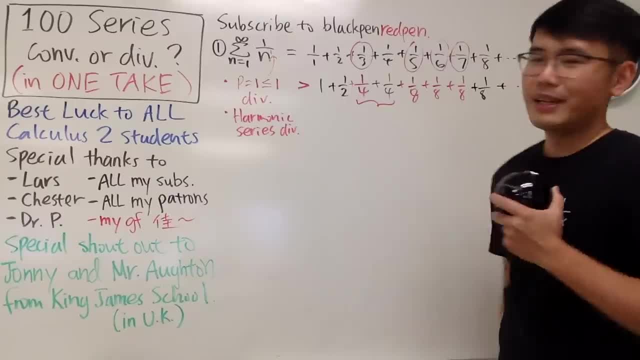 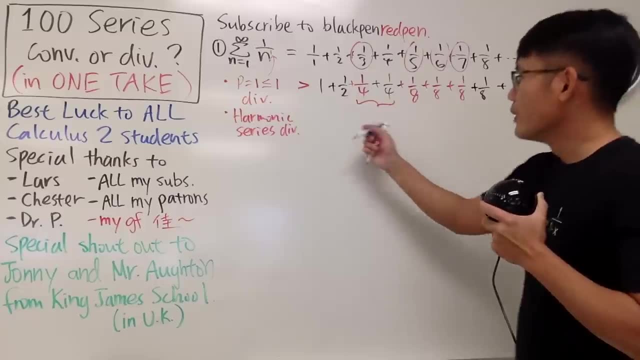 of doing so is that we can do more math fractions. 1 over 4 plus 1 over 4 is 2 over 4.. In another word, 1 half right. So the truth is this is equal to the following: 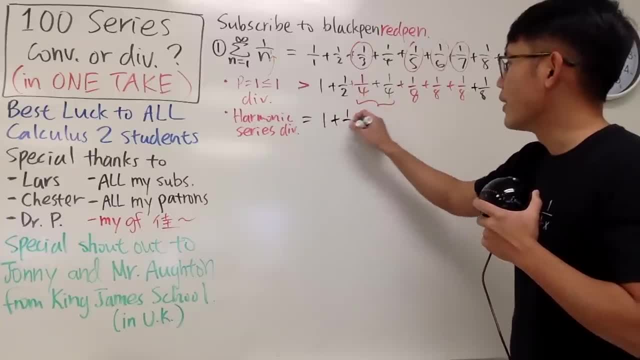 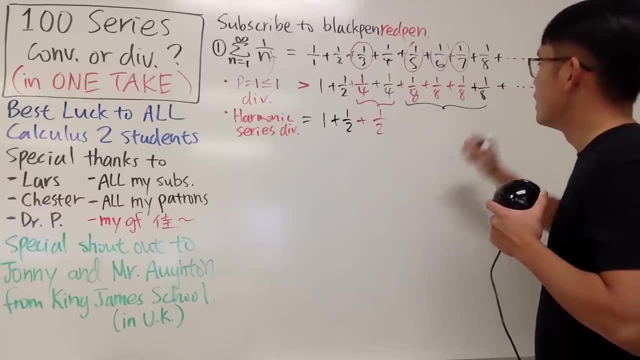 and we see that this is just 1 plus 1 half, and together this is just 1 half. And the next, all these four terms here: 1 over 8 plus 1 over 8 plus 1 over 8 plus 1 over 8. 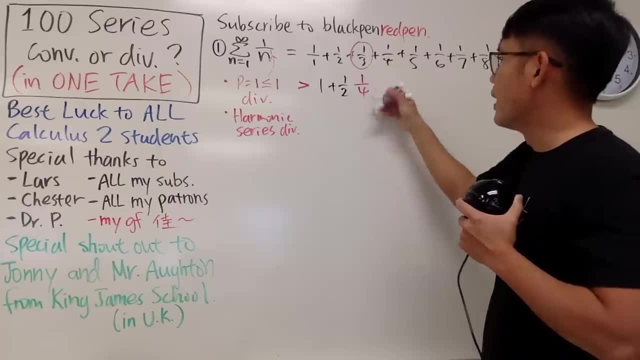 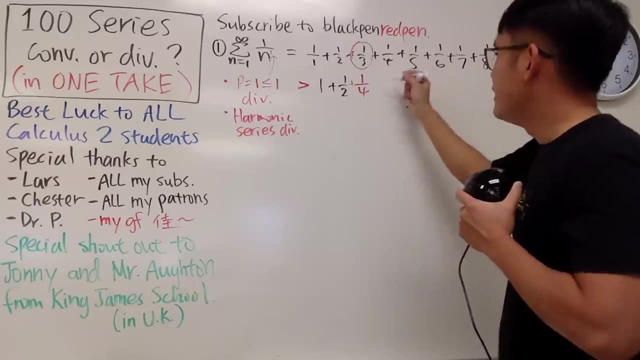 And then the 1 half. I will also keep that This is 1 over 4 now, But I'm saying this is greater than 1 over 4.. And of course I'll just put down plus And this 1 over 4 is still legit. 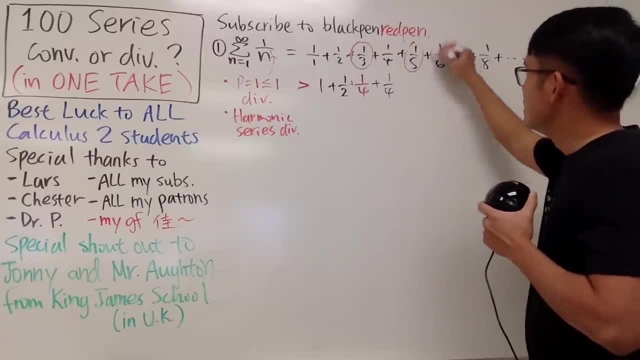 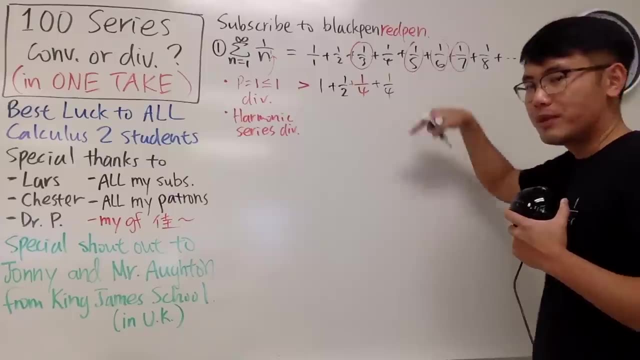 I'll just keep that down, And then for this, this and that, I will change them to 1 over 8. And of course, everybody here is bigger than 1 over 8.. So I will just put down: this is bigger than 1 over. 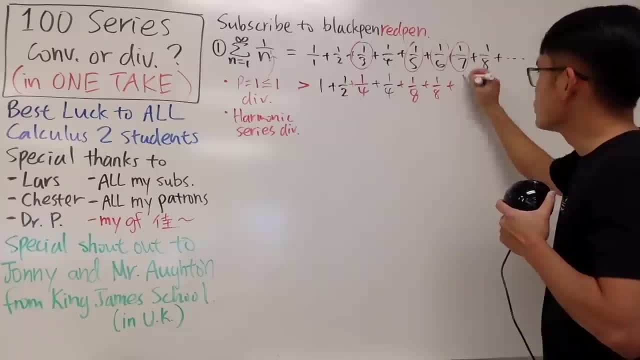 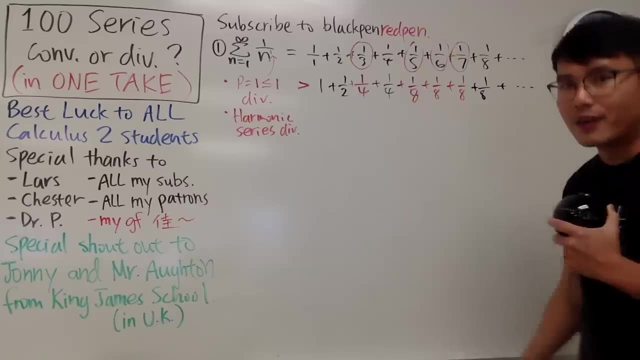 8. This is also bigger than 1 over 8.. And this is also bigger than 1 over 8.. And this is the 1 over 8 itself. And then, of course, this right here keeps on going forever. Now, the beauty. 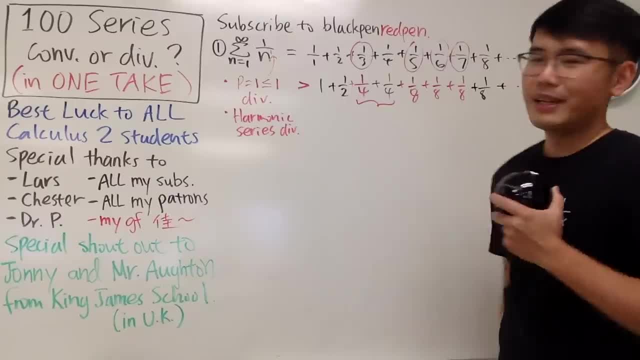 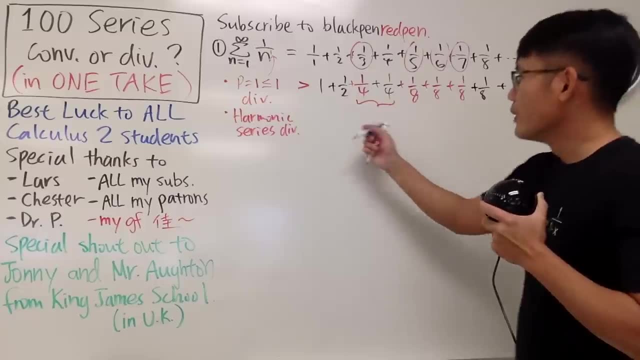 of doing so is that we can do more math fractions. 1 over 4 plus 1 over 4 is 2 over 4.. In another word, 1 half right. So the truth is this is equal to the following: 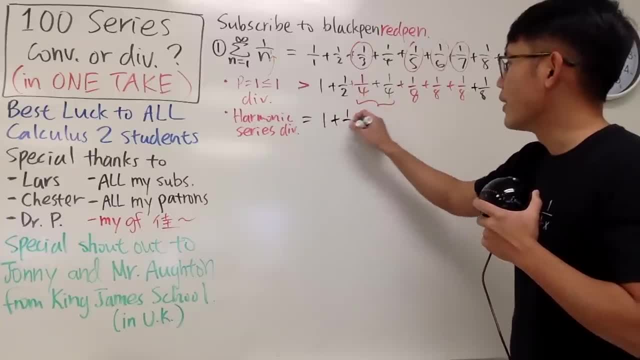 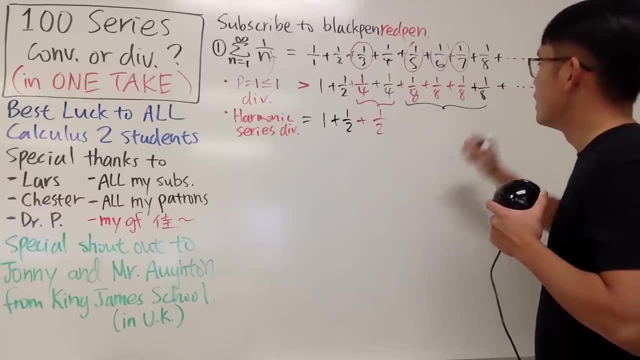 and we see that this is just 1 plus 1 half, and together this is just 1 half. And then next all these 4 terms here: 1 over 8 plus 1 over 8 plus 1 over 8 plus 1 over 8. 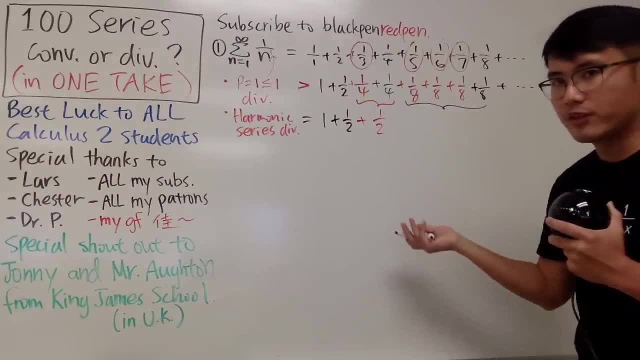 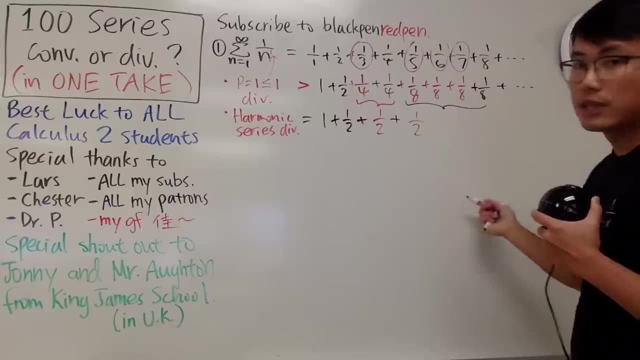 is 4 over 8.. Of course, that's 1 over 2 as well. So I will just say we can put down plus and all these guys is just 1 over 2 as well, And I just didn't put down the rest. but 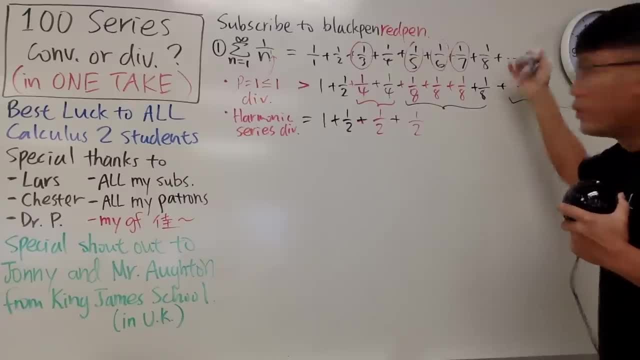 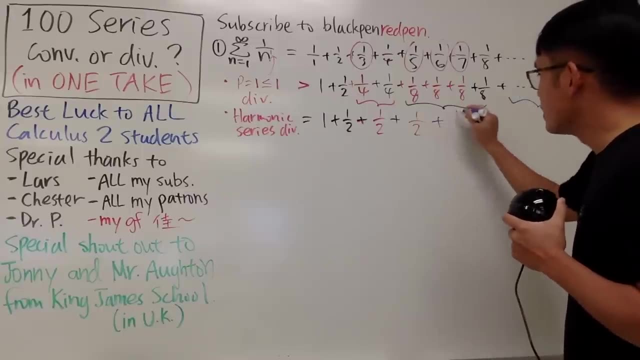 the idea is that if you continue with 1 over 9 here up to 1 over 16, you can also produce another 1 over 2.. So I will just put down another 1 over 2 right here for you guys. 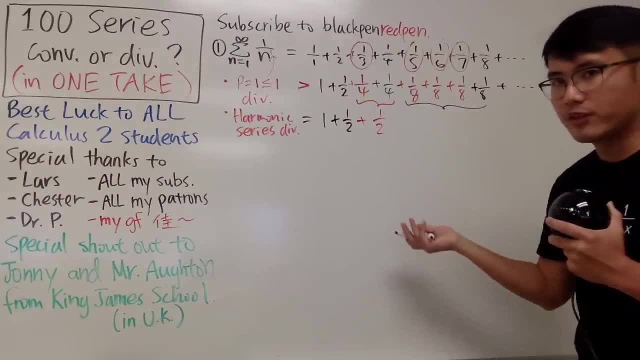 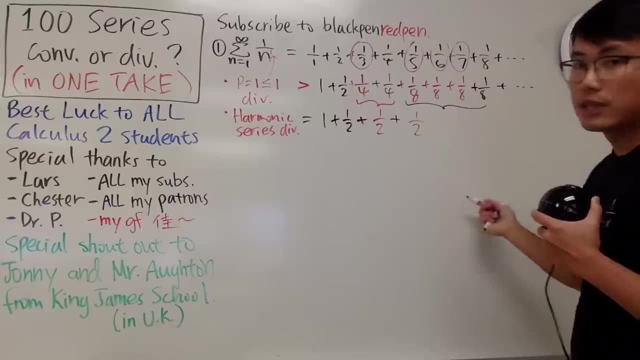 is 4 over 8.. Of course, that's 1 over 2 as well. So I will just say we can put down plus and all these guys is just 1 over 2 as well, And I just didn't put down the rest. but 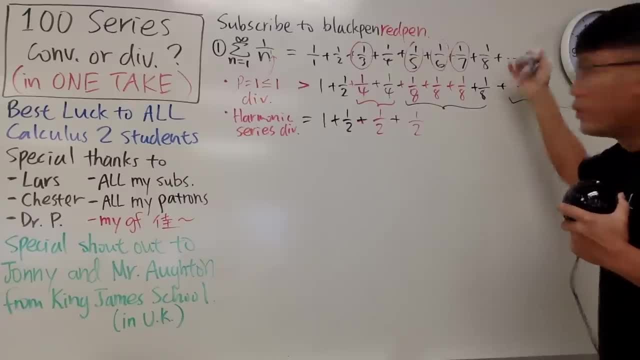 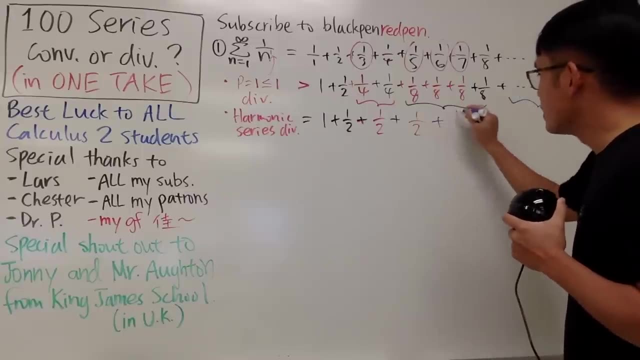 the idea is that if you continue with 1 over 9 here up to 1 over 16, you can also produce another 1 over 2.. So I will just put down another 1 over 2 right here for you guys. 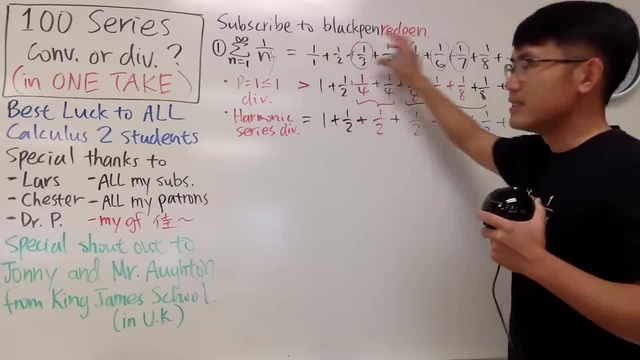 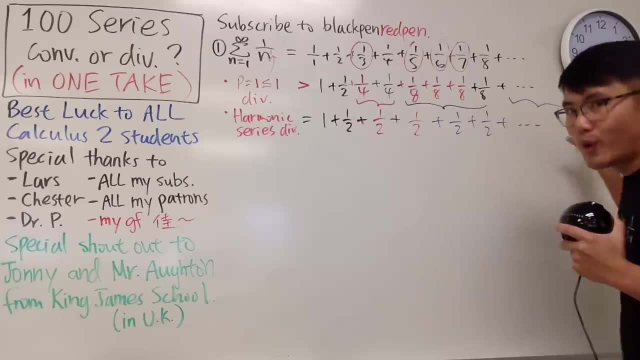 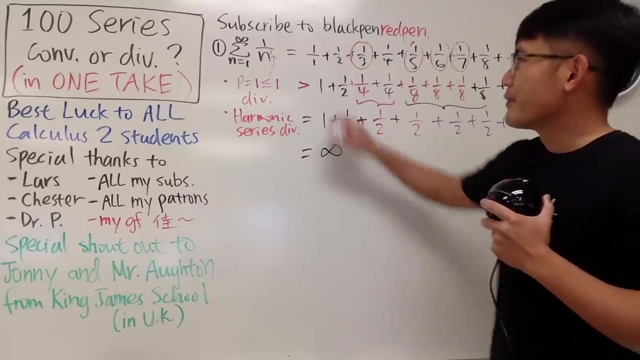 And notice that the truth is, this expression is bigger than this And this right here is 1 plus infinitely many 1 half. Of course, this right here is equal to infinity, or you can put down arrow up to you, So you can. 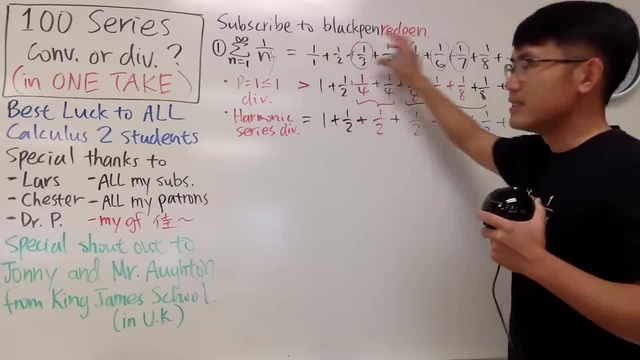 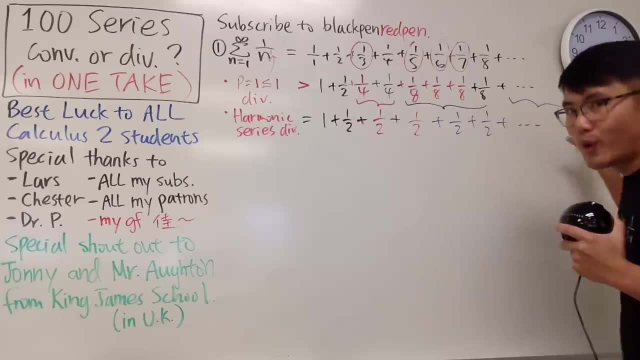 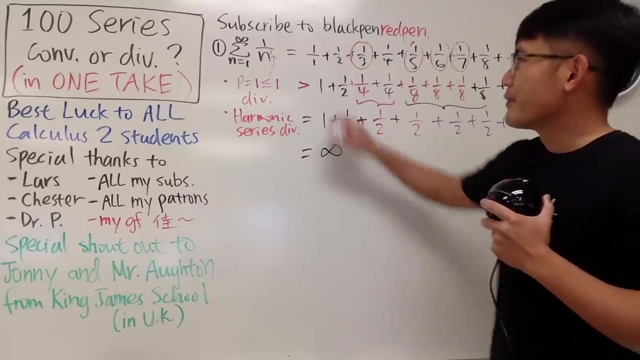 And notice that the truth is, this expression is bigger than this, And this right here is 1 plus infinitely many 1 half. Of course, this right here is equal to infinity, or you can put down an arrow, up to you, So you can. 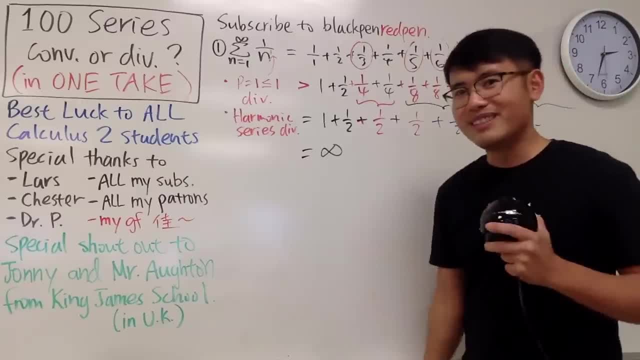 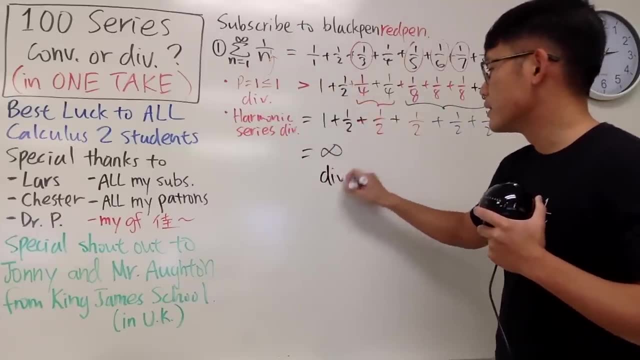 see that this right here is bigger than infinity. It has to be infinity. It's just a bigger version. right, Depends on how you want to write it. All in all this right here diverges. All in all this right here, the harmonic. 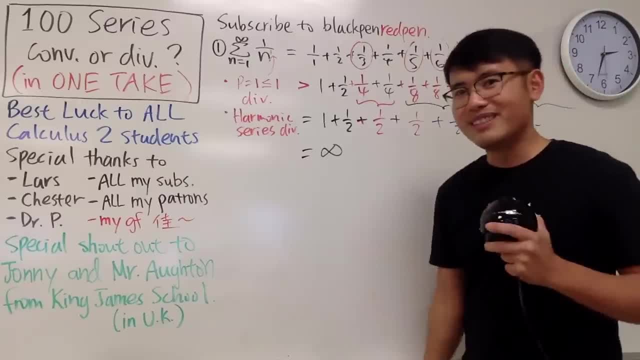 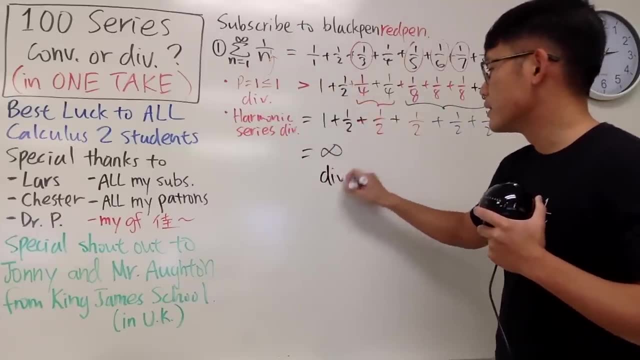 see that this right here is bigger than infinity. It has to be infinity. It's just a bigger version. right, Depends on how you want to write it. All in all this right here diverges. All in all this right here, the harmonic. 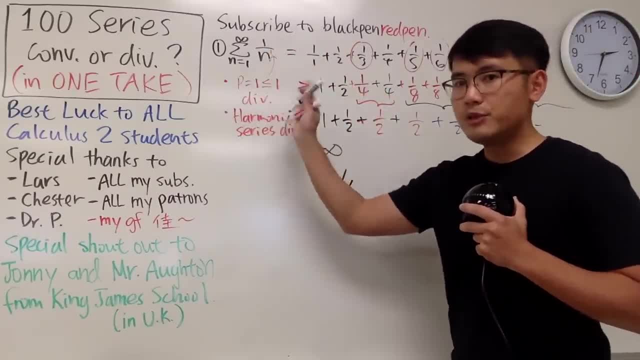 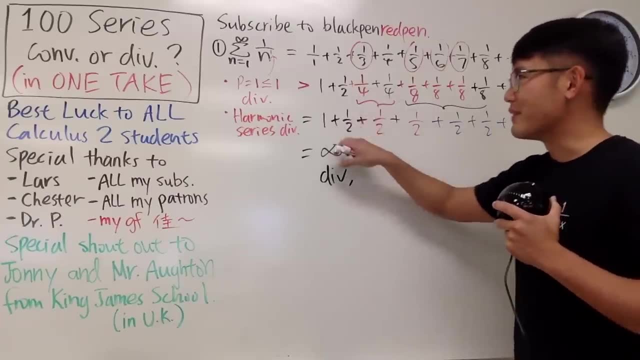 series diverges, And later on I will be using this, the p-series test, for that. But this is the classic proof: 1 plus infinitely many, 1 half is infinity, So that's why this diverges. This is bigger than. 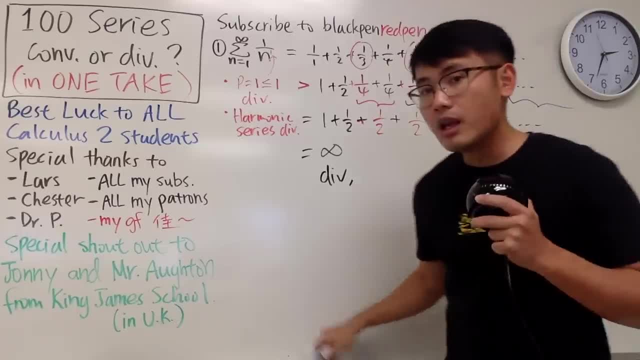 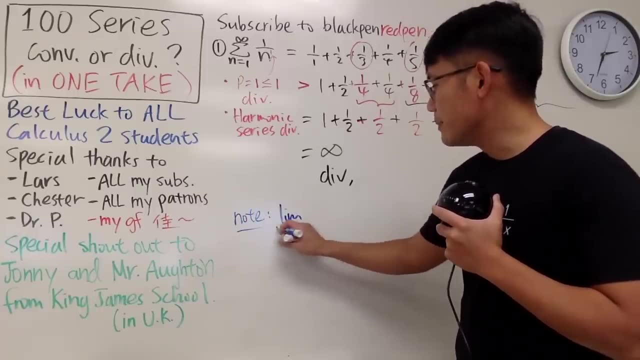 that. so that diverges as well. So that's the deal. Before we continue, I want to point out that notice right, even though if you take the limit as n goes to infinity of 1 over n, this right here. 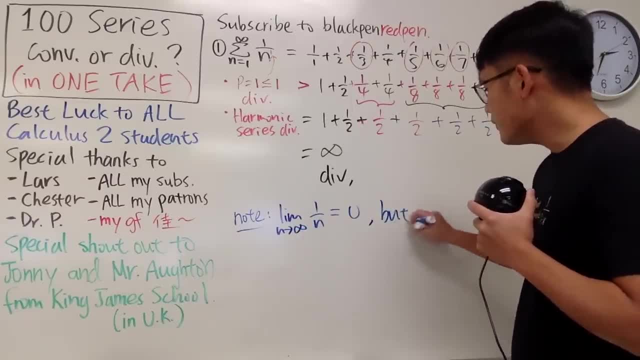 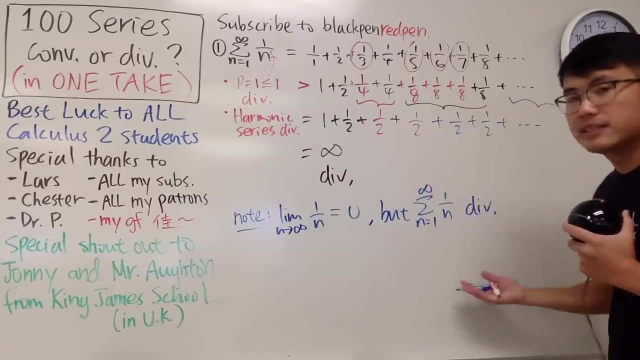 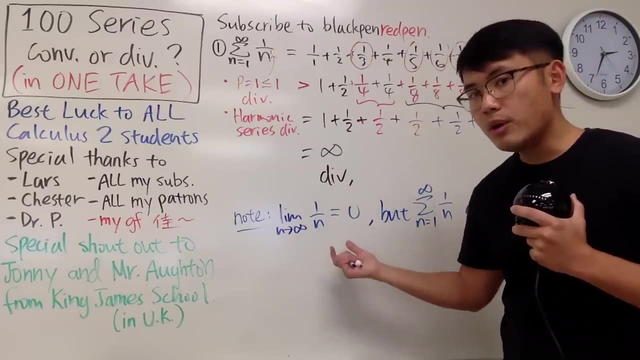 gives you 0,. but if you take the sum as n goes from 1 to infinity, of 1 over n, this right here diverges Right. So this right here, even though the term approaches 0, but we cannot draw any conclusion because 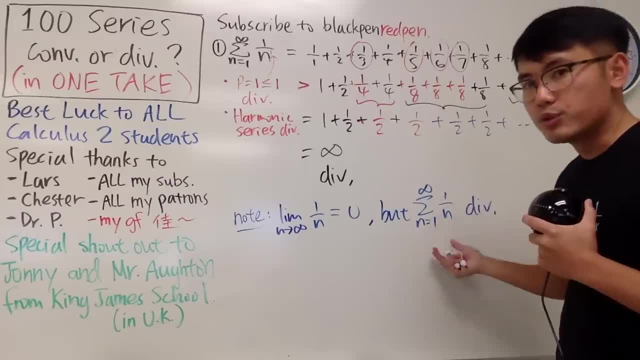 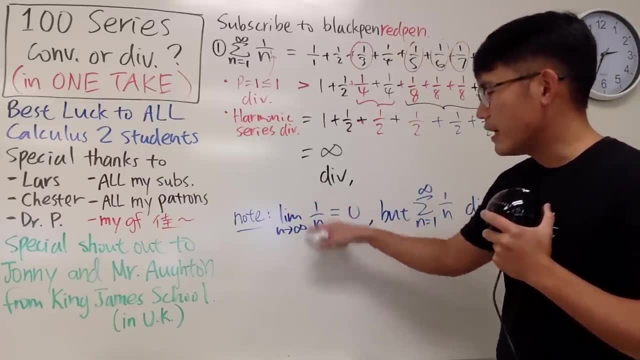 sometimes the sum of a n. if a n goes to 0, it may converge, it may diverge. This is an example that the sum of a n- sorry, the limit of a n- does go to 0, but the sum of a n. 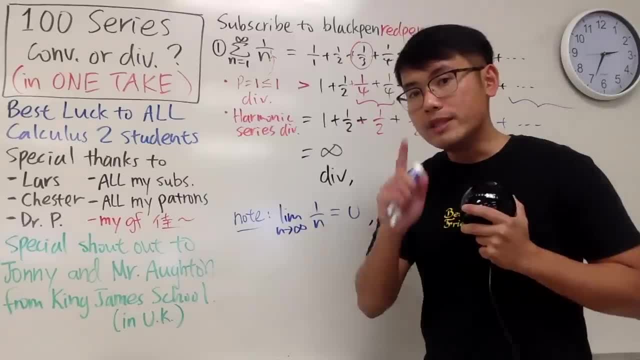 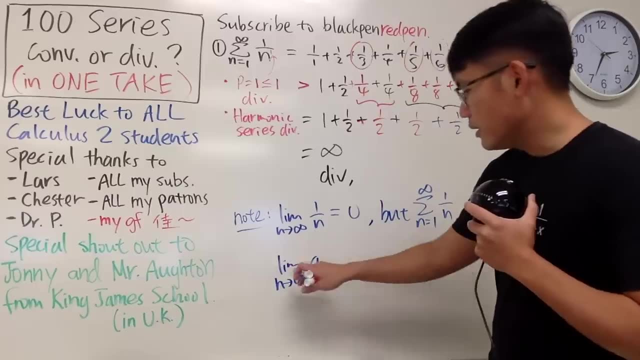 diverges Right. So that's the idea. One thing we can say, though: if, today, you have the limit as a n, as n goes to 0, the limit as n goes to infinity of a n, if this right here. 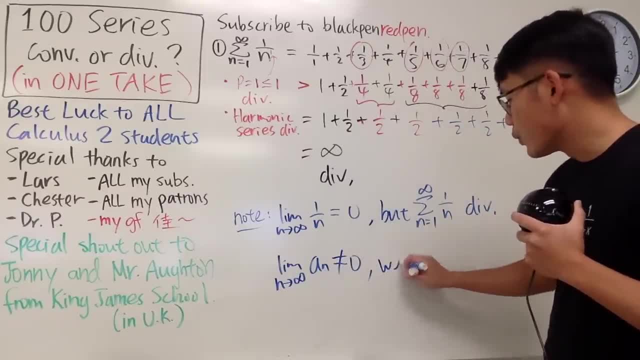 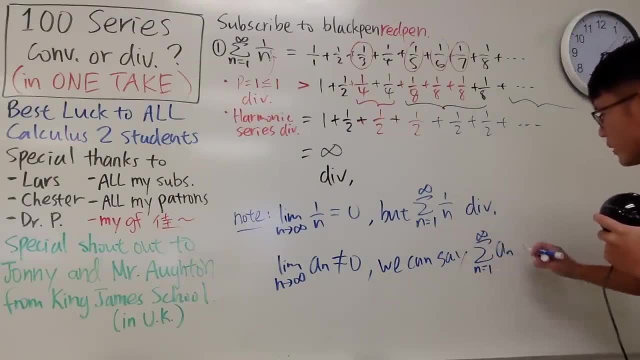 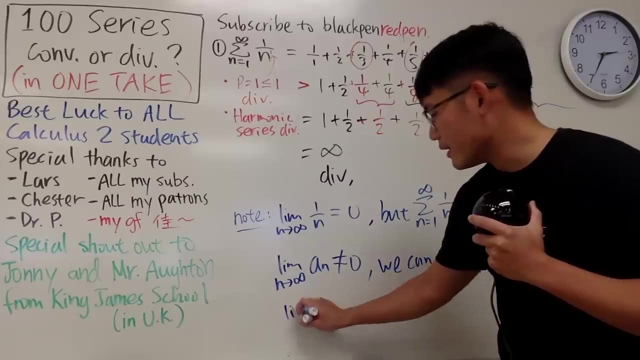 is not equal to 0, then we can say, we can say seriously, we can conclude that the sum of n goes from 1 to infinity of a n. this right here must diverge, Right Must diverge And if you have the limit, 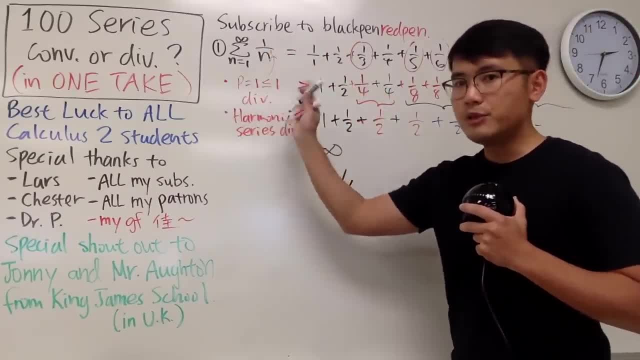 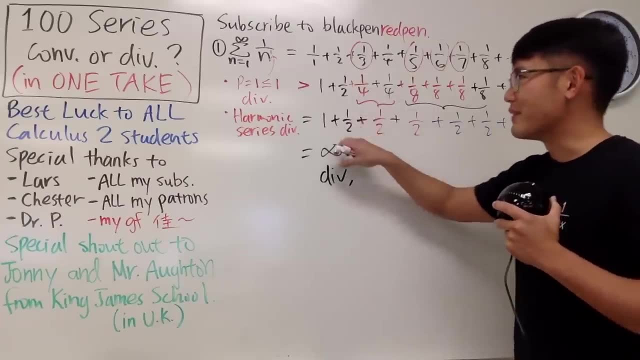 series diverges, and later on I will be using this, the p-series test, for that. But this is the classic proof: 1 plus infinitely many, 1 half is infinity, so that's why this diverges. This is bigger than that, so that diverges as well. 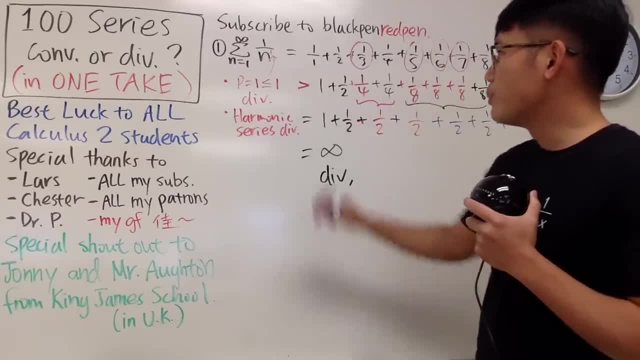 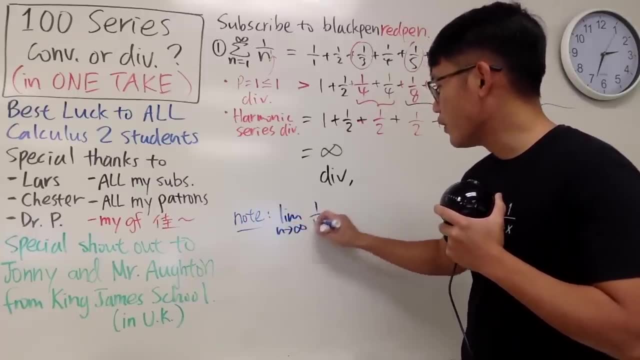 So that's the deal. Before we continue, I want to point out that. notice right: even though if you take the limit, as n goes to infinity, of 1 over n, this right here is give you 0 by 0. But if you take, 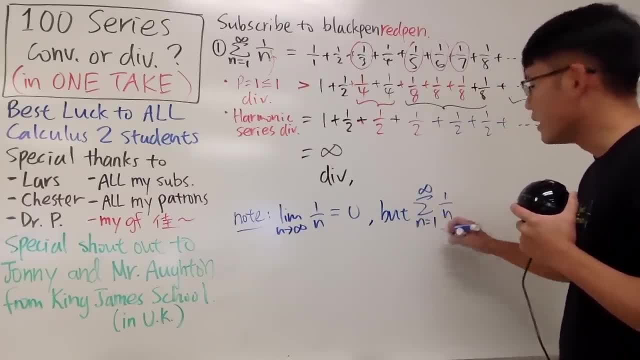 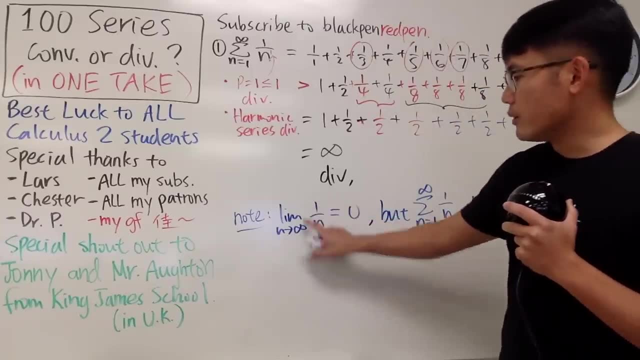 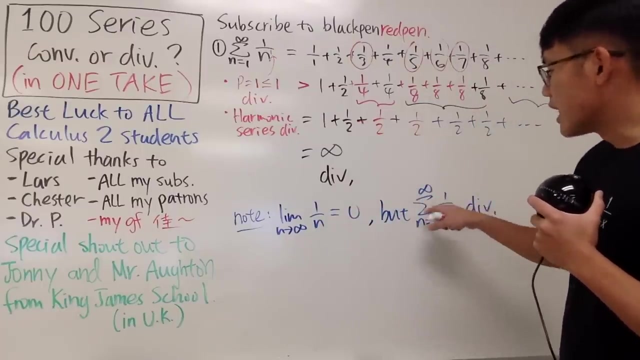 the sum as n goes from 1 to infinity, of 1 over n. this right here, diverges Right. So this right here, even though the term approaches 0,. but we cannot draw any conclusion because sometimes the sum of a n, if a n goes to 0,. 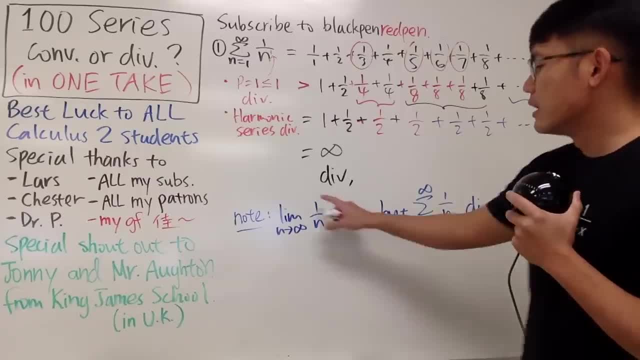 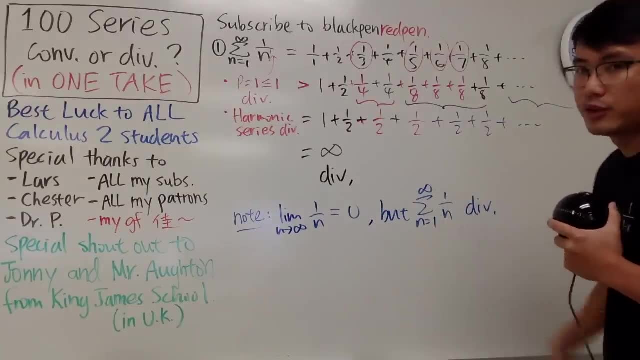 it may converge, it may diverge. This is an example that the sum of a n- sorry, the limit of a n- does go to 0, but the sum of a n diverges, Right. So that's the idea, One thing we can. 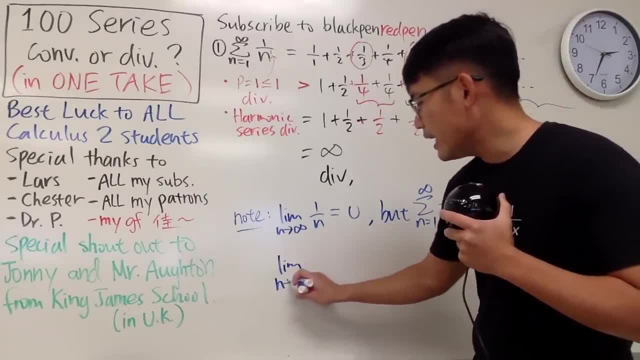 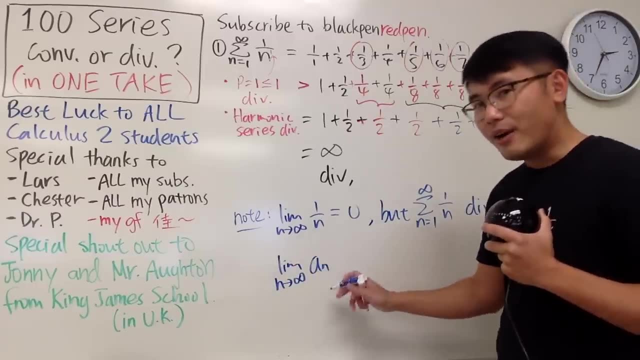 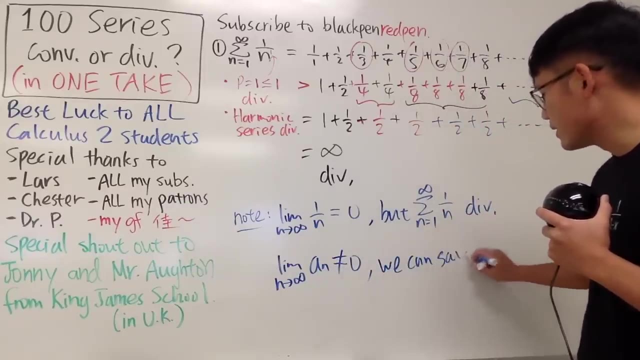 say though: if today you have the limit as a n, as n goes to 0, the limit as n goes to infinity of a n, if this right here is not equal to 0,, then we can say, we can say seriously, we can conclude: 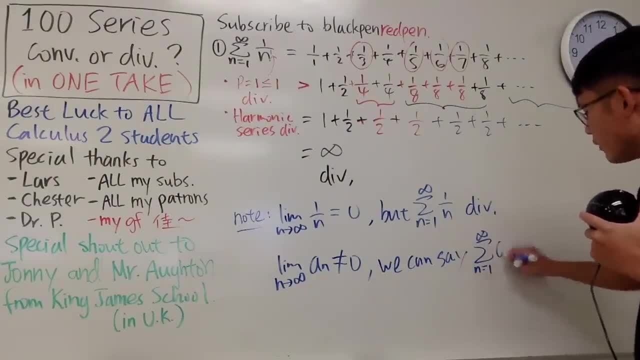 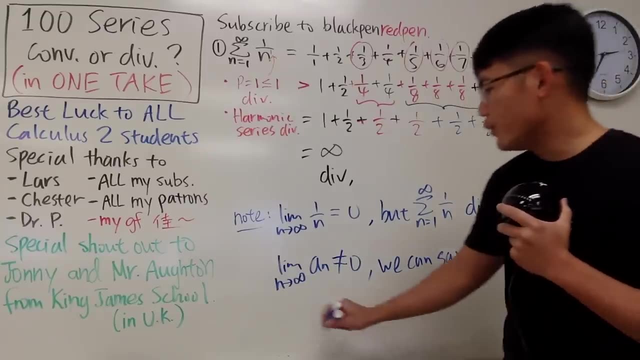 that the sum of n goes from 1 to infinity of a n. this right here must diverge, Right Must diverge. And if you have the limit as n goes to infinity of a n, if this happens to be 0,. 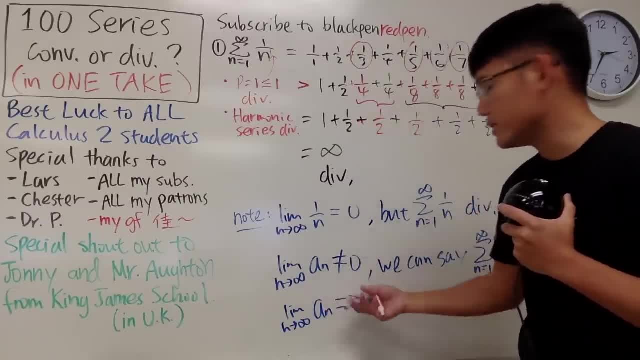 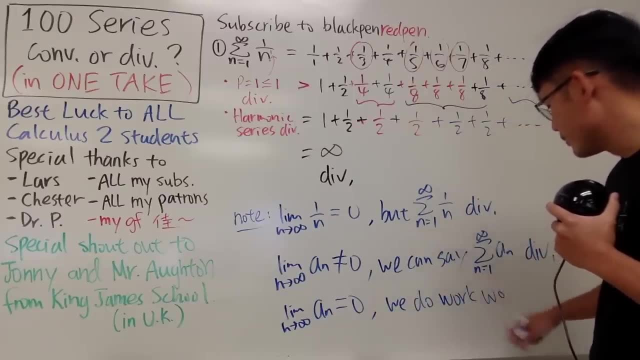 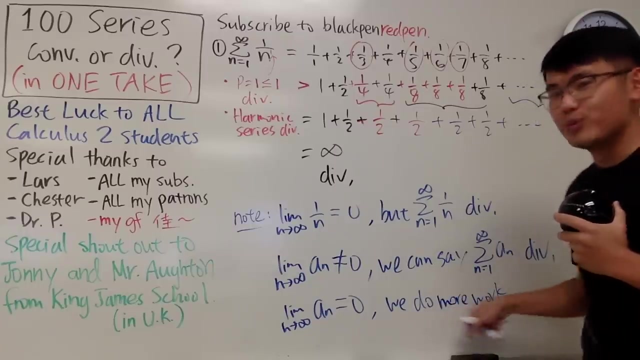 as n goes to infinity of a n. if this happens to be 0,, then we have to do more work, We do more, We do work, We do more work, Right? So that's the idea, And of course, do not just put down: do more work. 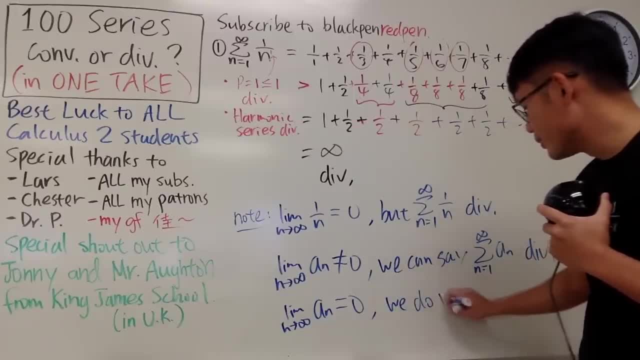 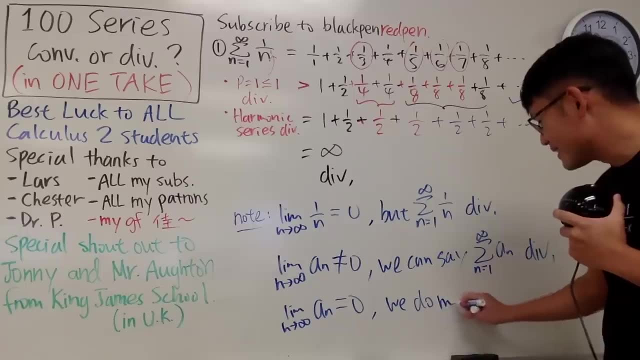 then we have to do more work, We do more, We do work, We do more work. Right, So that's the idea. And, of course, do not just put down: do more work on the test. you really have to do more work to convince. 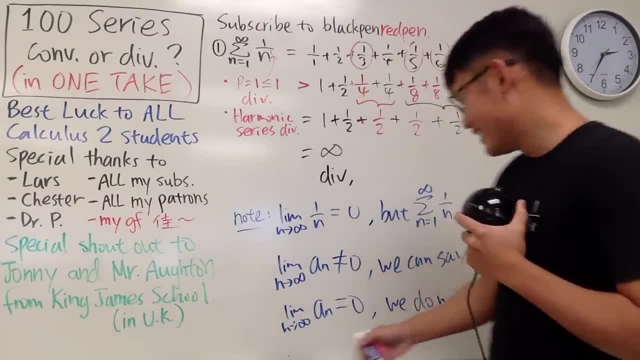 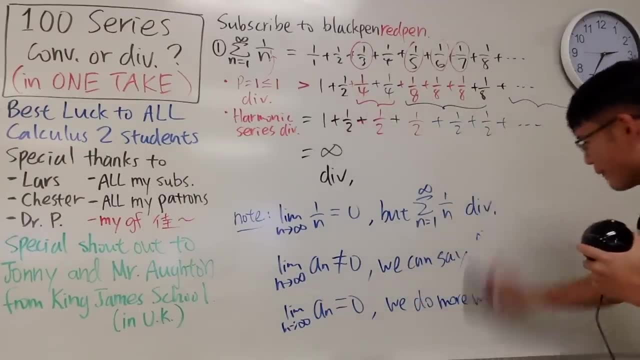 people that it's actually convergent or it's actually divergent, Right? So that's the idea. So that's it, And we have 99 more to go. Alright, So here we go. We're just going to erase all the board and then 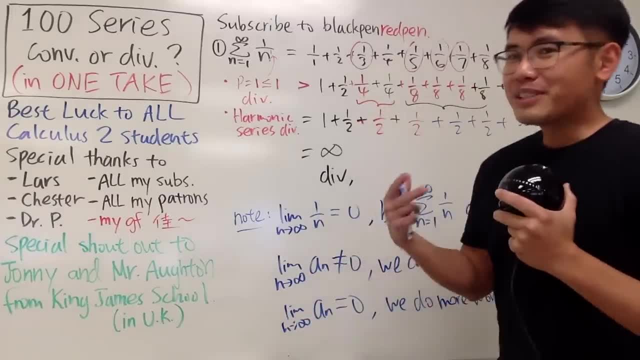 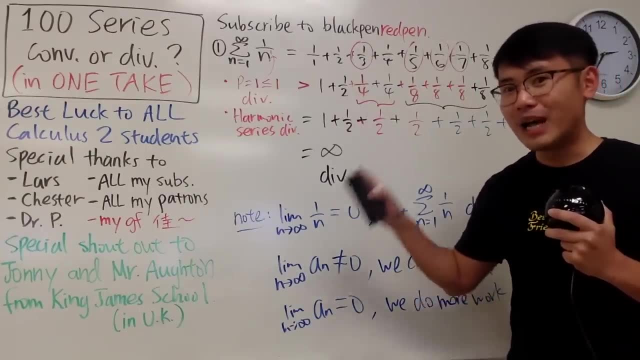 on the test. You really have to do more work to convince people that it's actually convergent or it's actually divergent, Right? So that's the idea. So that's it, And we have 99 more to go. 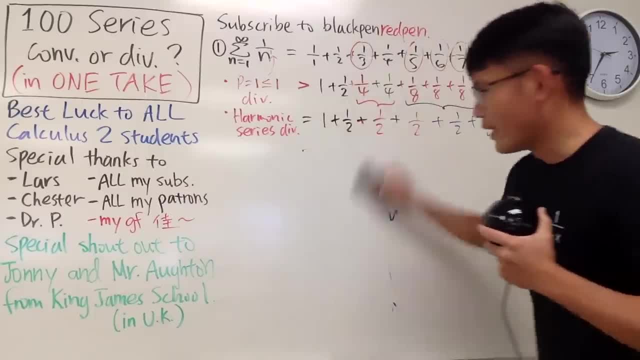 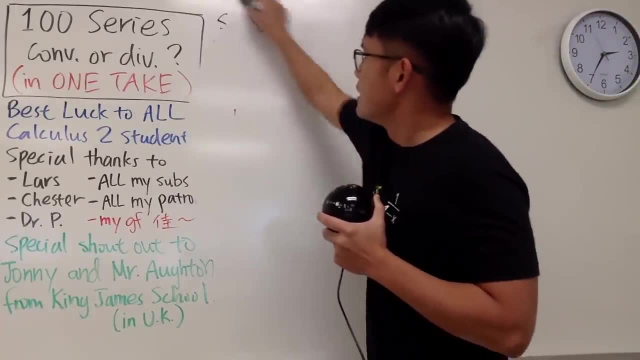 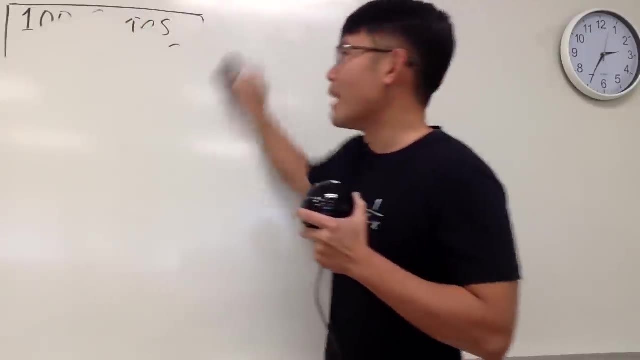 Alright, So here we go. We're just going to erase all the board and then see what happens. Of course, whatever happens happens, Yeah. So let me know, Leave a comment, let me know what final exams that you guys have coming up. 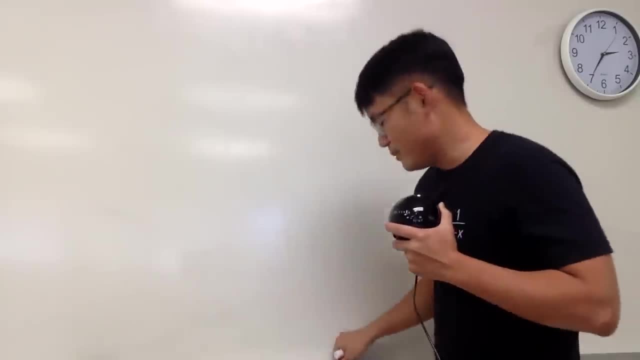 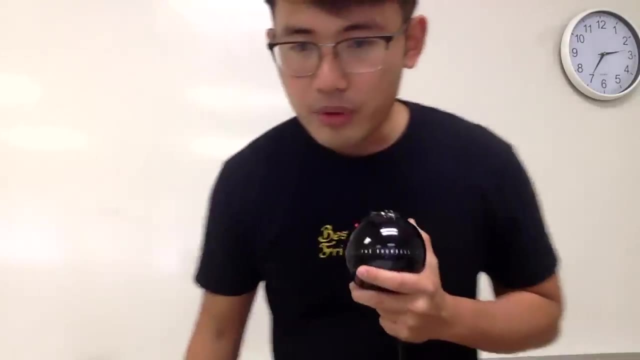 So I can wish you guys good luck. If you are not taking Cal 2, let me know what else you are taking. Or maybe you are just enjoying the math, And in that case that would be cool as well. Okay, Continue Number 2.. We are going. 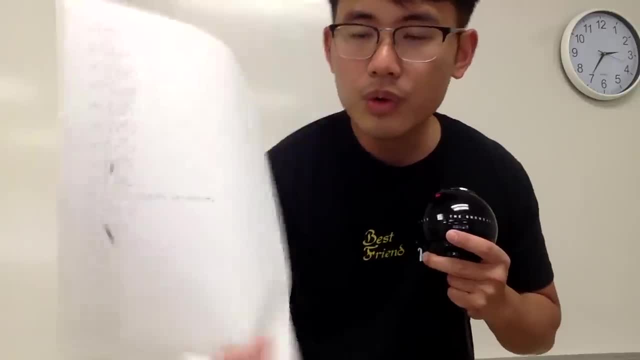 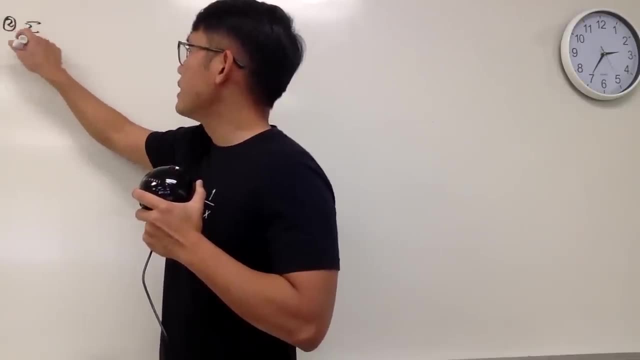 to take care of the sum as n goes from 2 to infinity of natural log of n. So let me write this down right here For you guys: the sum as n goes from 1, sorry, goes from 2 to infinity. 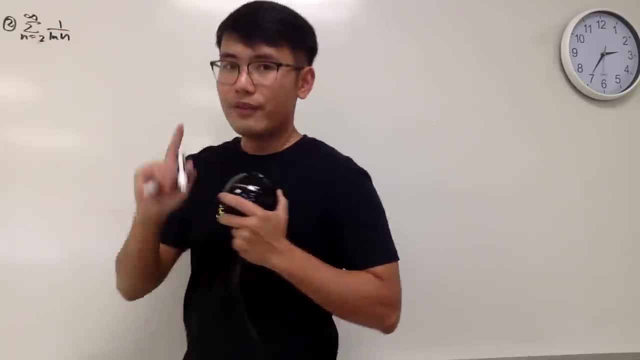 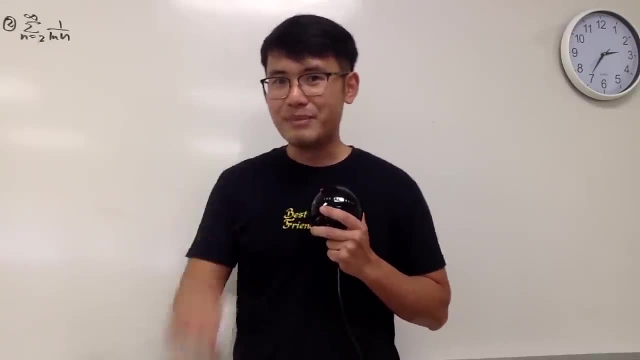 of 1 over natural log of n. First of all, leave a comment down below and let me know why don't we start with n equals 1, but rather we are doing this from 2 to infinity. Let me know, Alright. 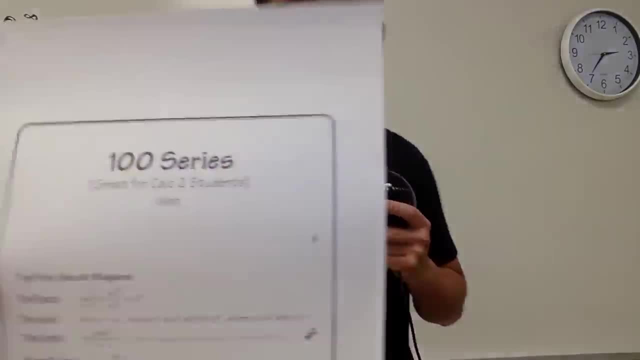 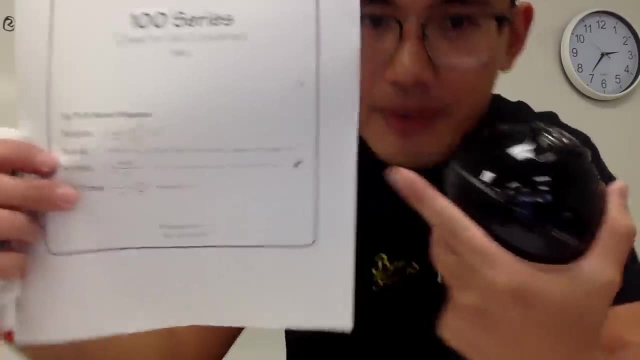 Here is the deal. You have to keep the list in your mind, Right? This is how we can compare the kind of infinity right here, Right, As you all know, ln n is the smallest infinity. So let me just write this: 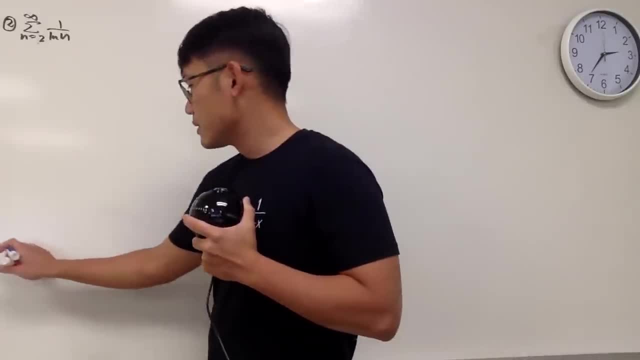 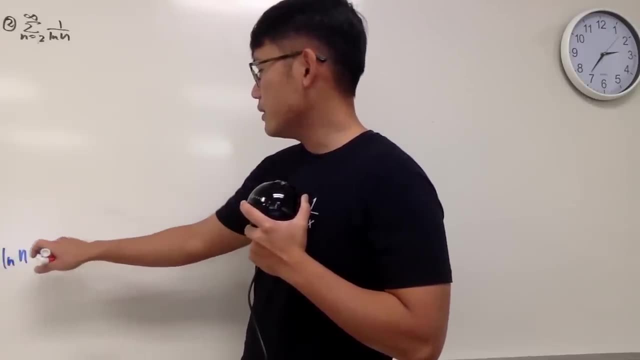 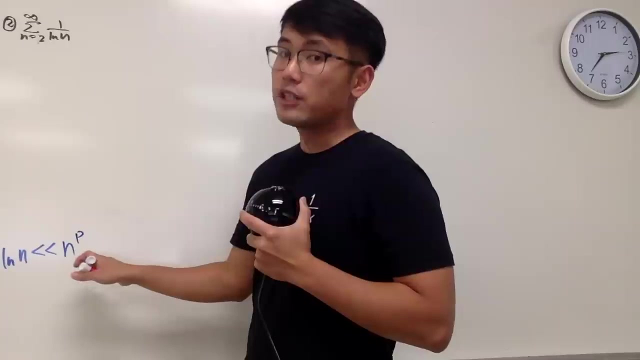 down right here for you guys. So this is the list. ln n is the smallest kind of infinity And so small and it's going to be 0 if you do a ratio of ln n with other things right here. But anyway, this is the first part that you have to. 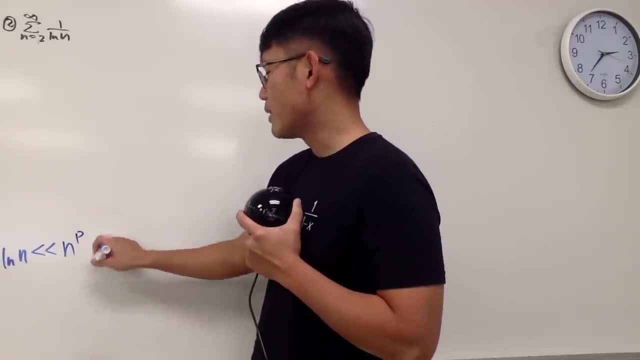 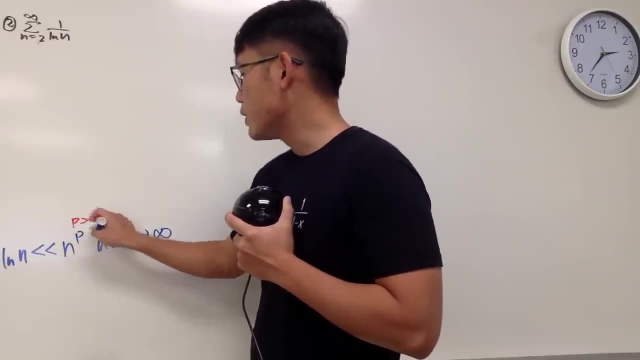 know, ln, n is less than or less than n to the p's power, as n goes to infinity Right And of course in this case the p has to be greater than 0, some positive exponent, And we can also talk about the. 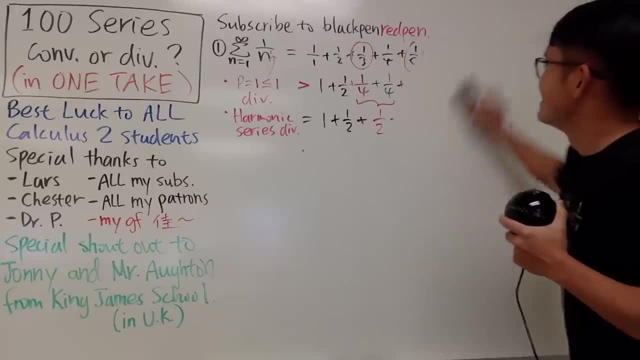 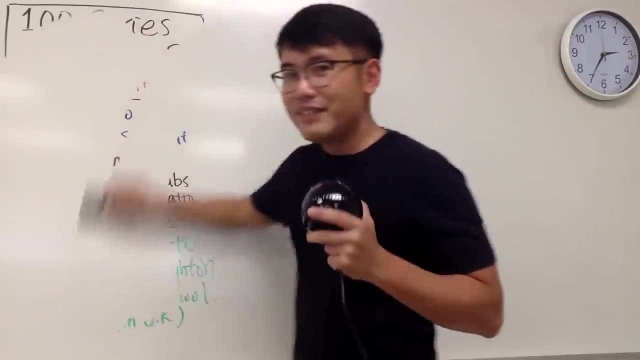 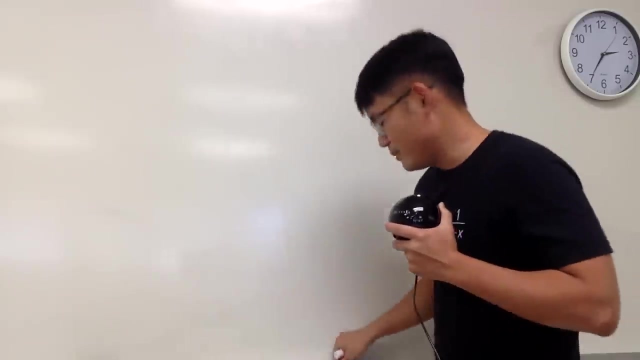 see what happens. Of course, whatever happens happens, Yeah. So let me know, Leave a comment, let me know what final exams that you guys have coming up So I can wish you guys good luck. If you are not taking Cal 2, let me know. 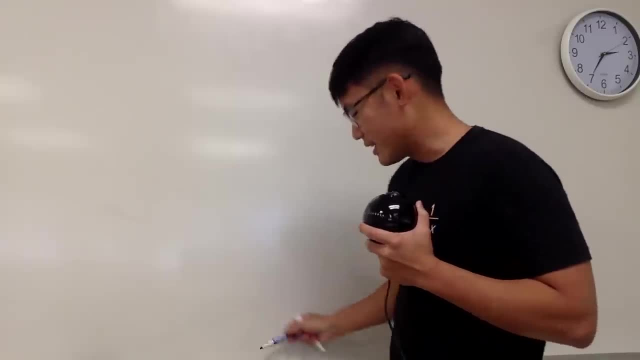 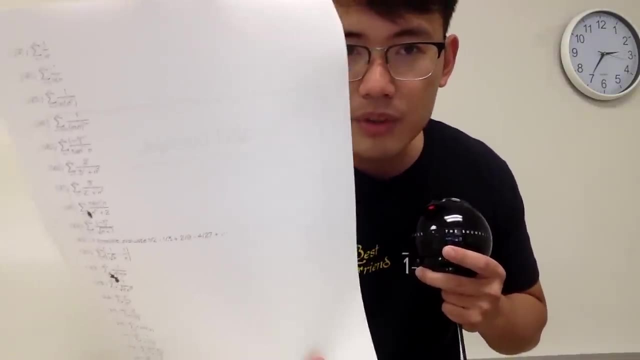 what else you are taking, Or maybe you are just enjoying the math, And in that case that would be cool as well. Okay, Continue Number 2,. we are going to take care of the sum as n goes from 2 to infinity. 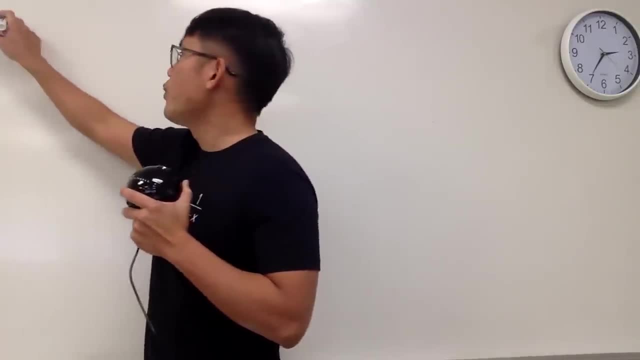 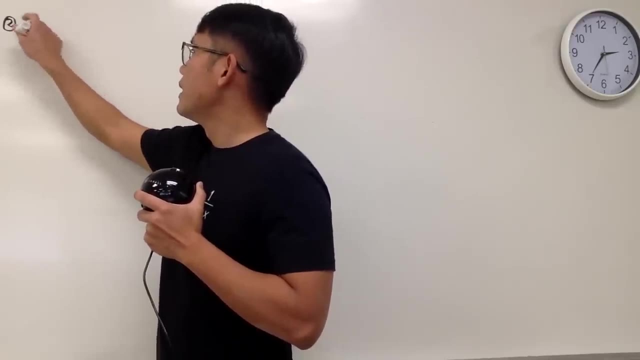 of natural log of n. So let me write this down right here For you guys: the sum as n goes from 1, sorry, goes from 2 to infinity of 1 over natural log of n. First of all, leave a comment down below and let me know why don't. 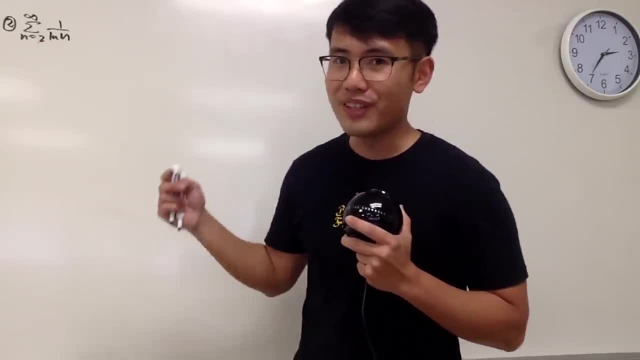 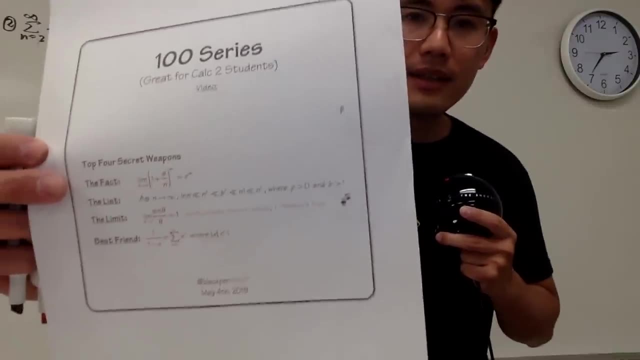 we start with n equals 1, but rather we are doing this from 2 to infinity. Let me know. Alright, here is the deal. You have to keep the list in your mind, Right? This is how we can compare the kind of infinity, right here? 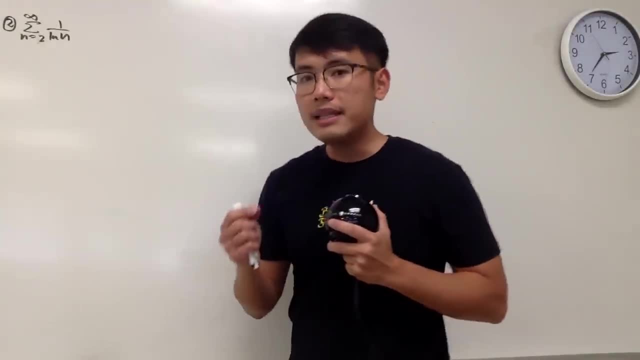 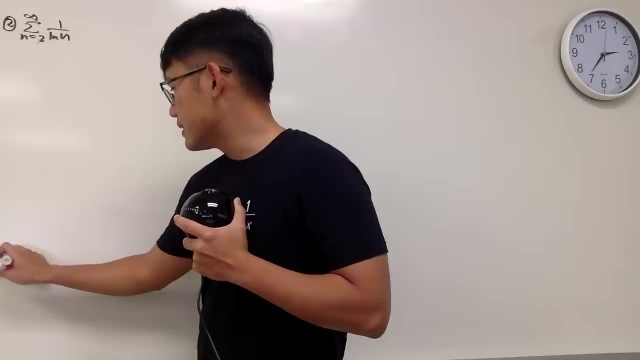 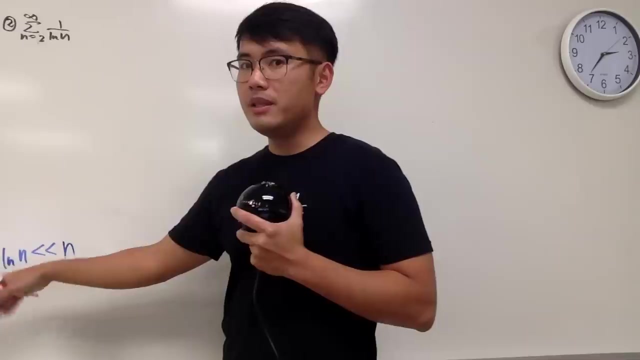 Right, As you all know, ln n is the smallest infinity, So let me just write this down right here for you guys. So this is the list: ln n is the smallest kind of infinity And so small and it's going to be. 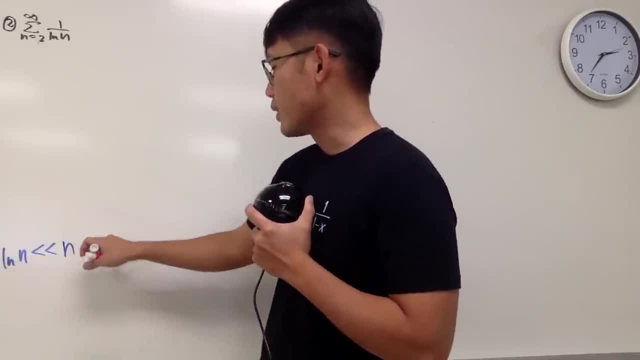 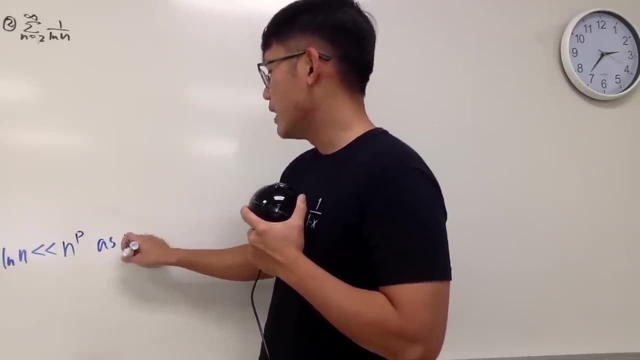 0 if you do a ratio of ln n with other things right here. But anyway, this is the first part that you have to know. ln n is less than or less than n to the p's power, as n goes to infinity Right And 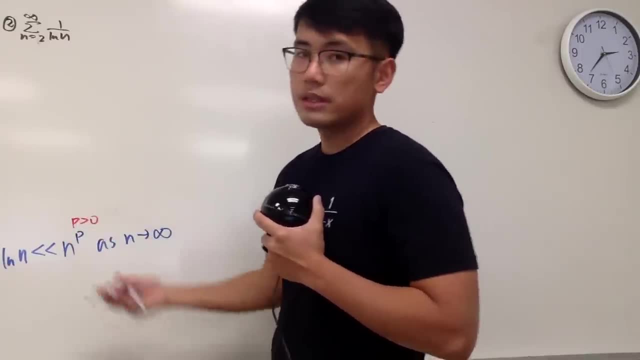 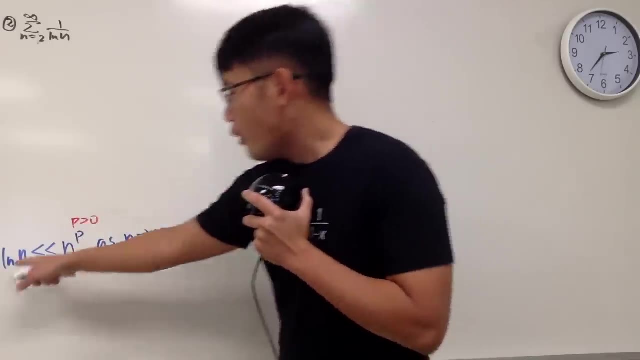 of course, in this case the p has to be greater than 0, some positive exponent. And we can also talk about the reciprocal version of this. Both terms, both of this, they are positive. So if you take the reciprocal, you have 1 over ln n. 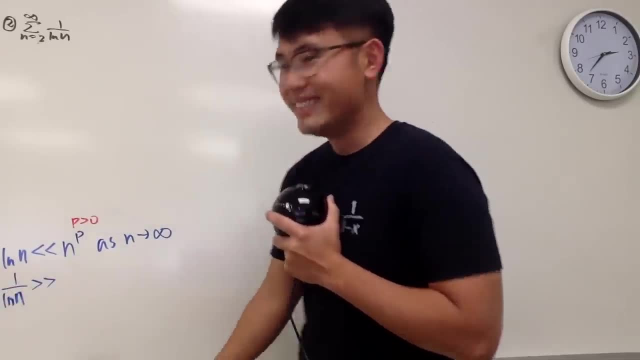 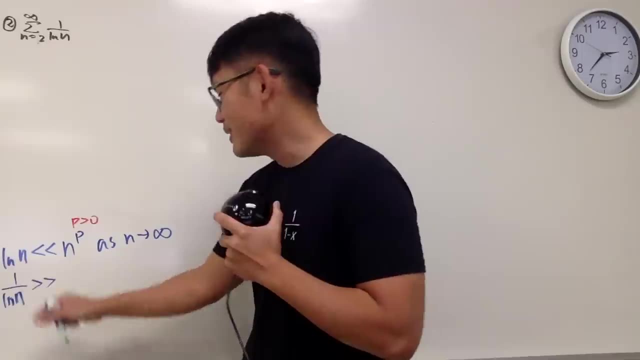 And this is going to be the biggest, the biggest 0 that you will get, because the bottom is infinity, Right, So 1 over infinity is 0. But this is going to be the biggest compared to 1 over n, to the p's power. Now, 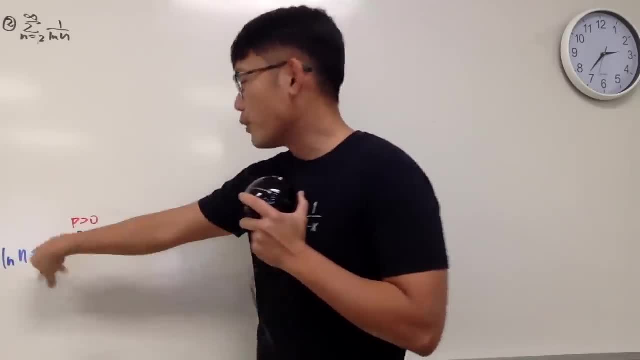 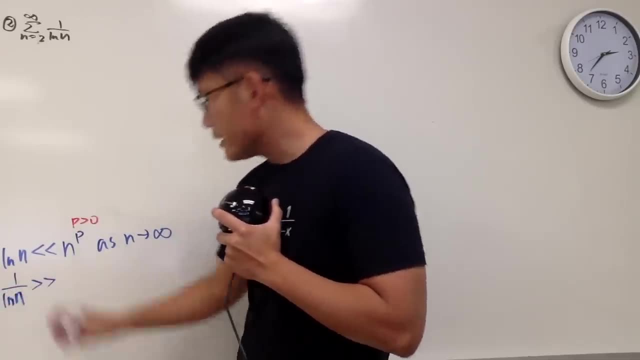 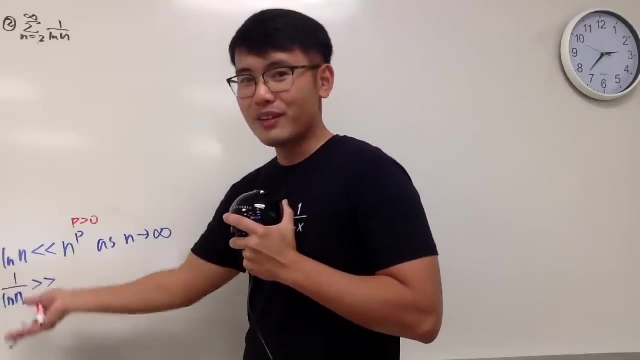 reciprocal version of this. Both terms, both of this, they are positive. So if you take the reciprocal, you have 1 over ln, n And this is going to be the biggest, the biggest 0 that you will get because the bottom is infinity, Right. So 1 over infinity. 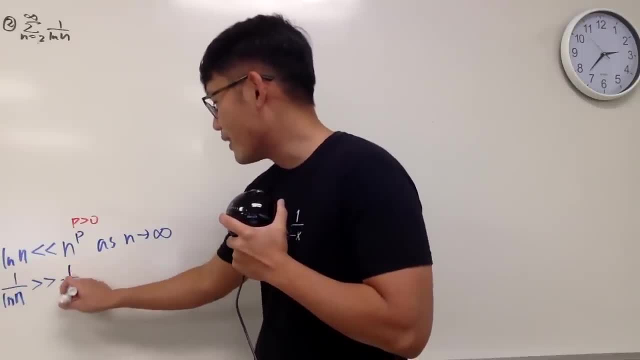 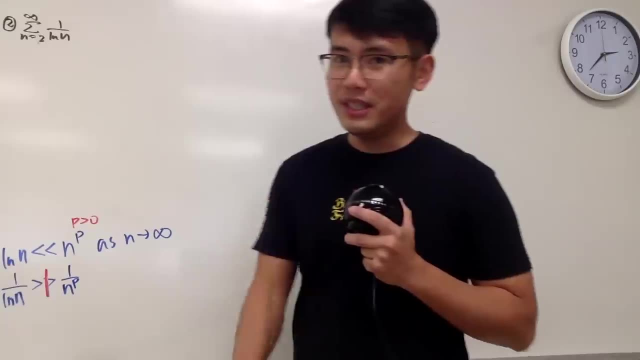 is 0. But this is going to be the biggest compared to 1 over n, to the p's power. Now here is the breaking point, Right, The one that we just did earlier. That's like the classic example of a divergent. 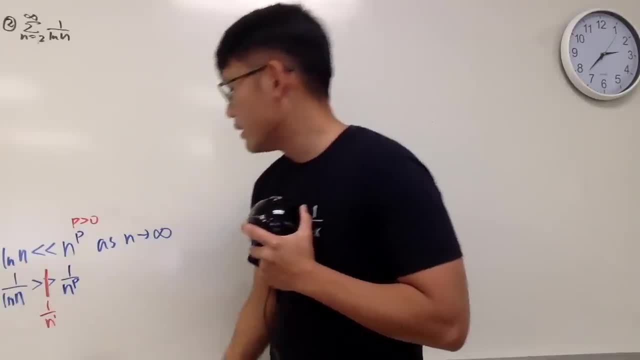 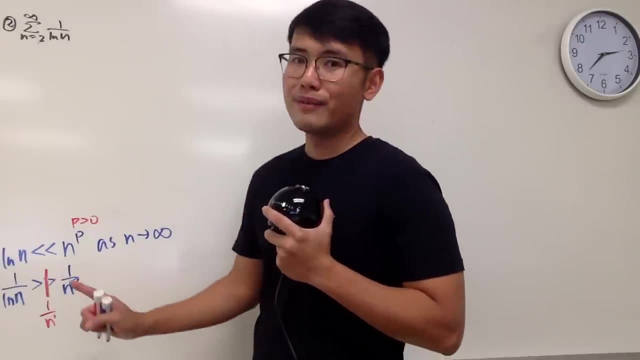 You have to pay attention to 1 over n to the first power. Of course, 1 over n to the first power is somewhere right here, when p is equal to 1.. Well, remember the p-series. if p is greater than 1, then that series. 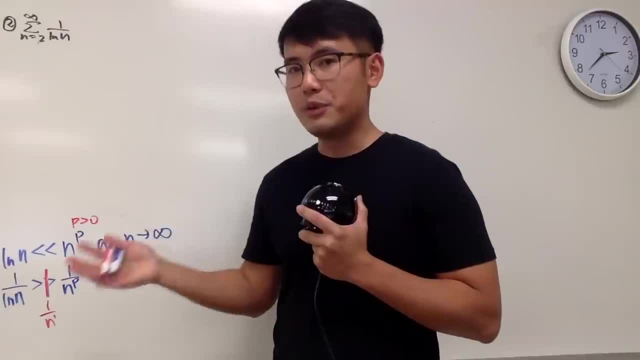 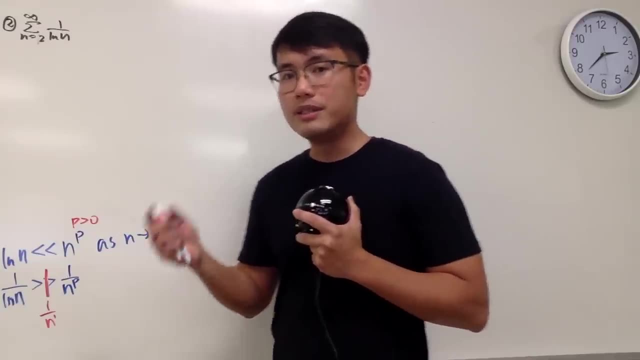 converges. If p is less than or equal to 1,, then that series diverges. If p is greater than 1, it converges, And if p is less than or equal to 1, the series diverges. Okay. 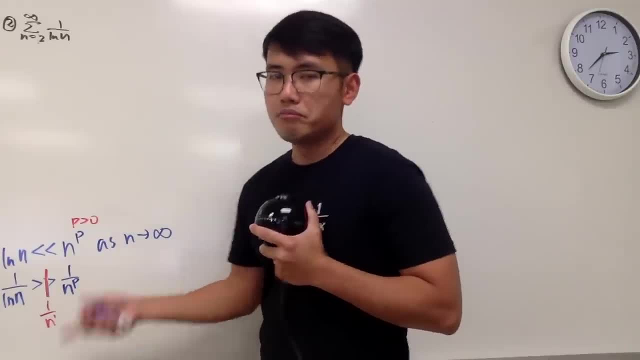 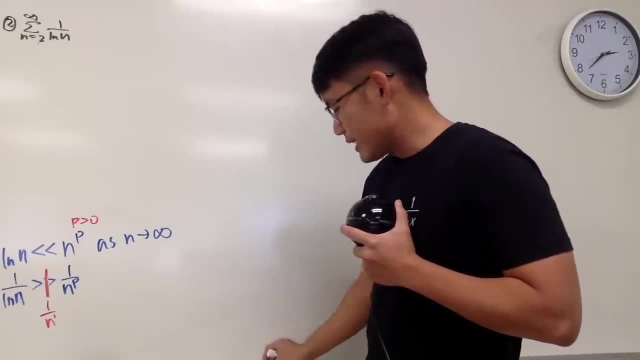 And then you can see that this is bigger than 1 over n. So of course you can see that this right here diverges by the list. So I will just show you guys how we can write this down the quicker way, right? So? 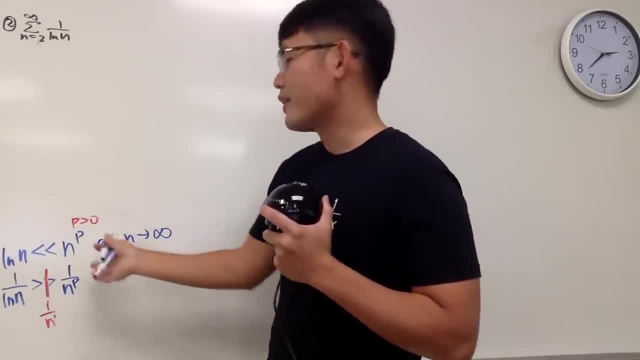 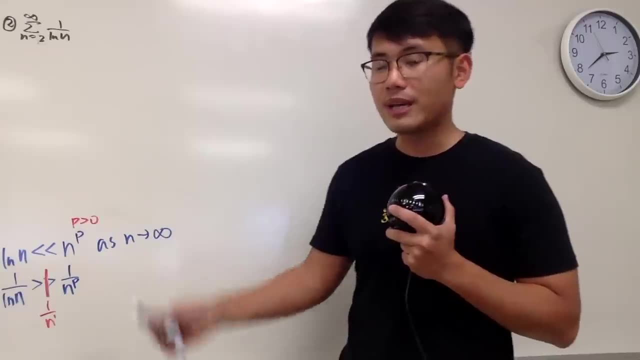 and, of course, it also depends on your teacher. This right here is something that I allow my students to just use, and I think it's good because they can compare the different kinds of infinity and all that. So the idea is that notice. 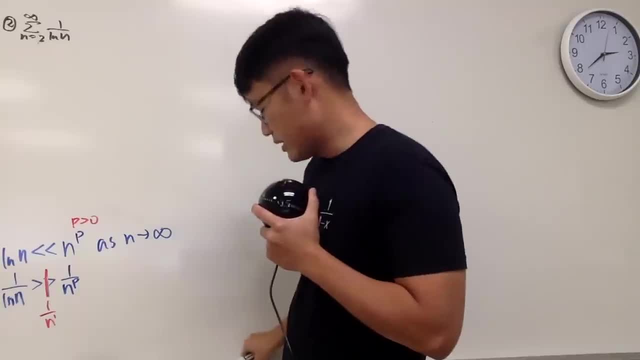 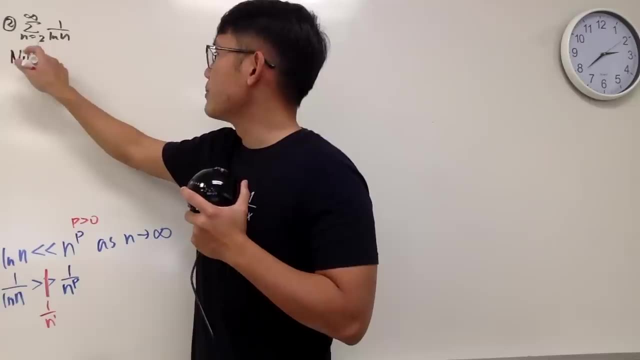 I'll just put down: this is how I will show work for you guys, right? So I will just say: note. well, note is up to you. however you want to say it. Note 1 over ln n is bigger than. 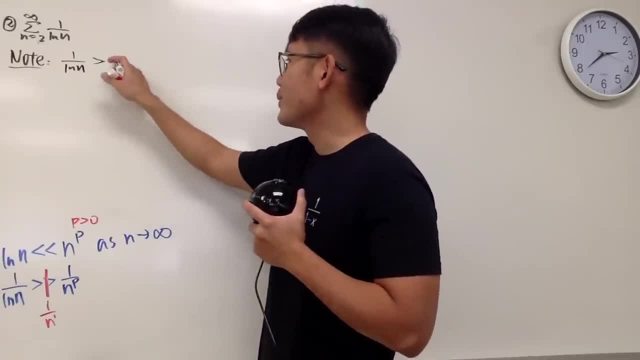 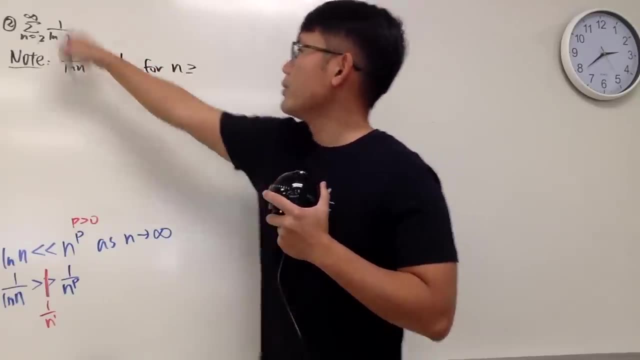 well, technically you don't have to put an equal sign, because it's not equal anyway: 1 over n to the first power. like this for n greater than or equal to 2, because we're going from 2 to infinity. So 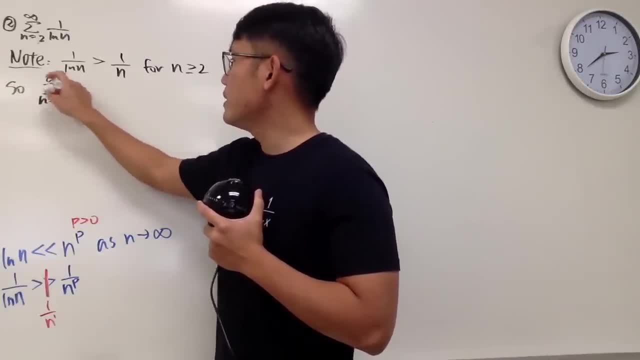 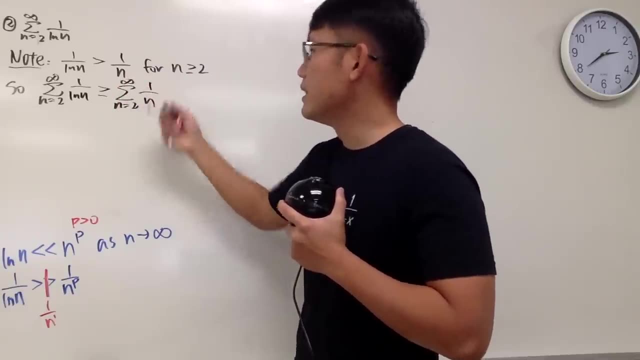 the sum as n goes from 2 to infinity of 1 over ln, n is greater than or equal to the sum as n goes from 2 to infinity of 1 over n, like this. And now check this out Earlier the example: 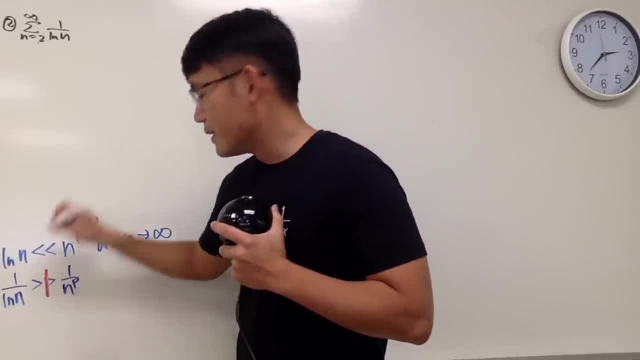 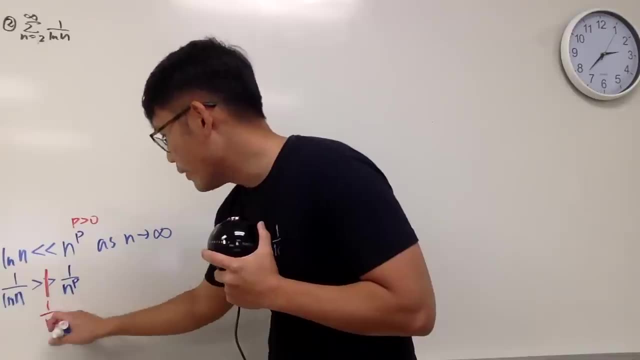 here is the breaking point, Right, The one that we just did earlier. that's like the classic example of a divergent You have to pay attention to 1 over n to the first power. of course 1 over n to the first power is. 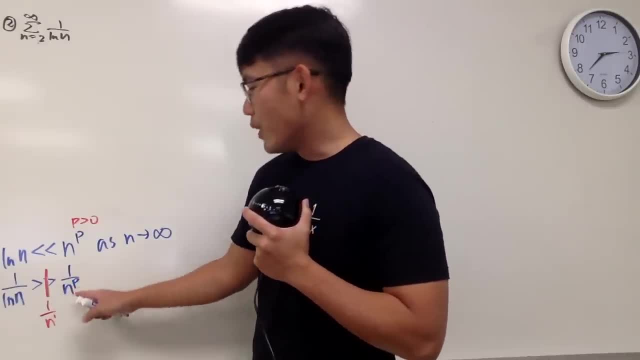 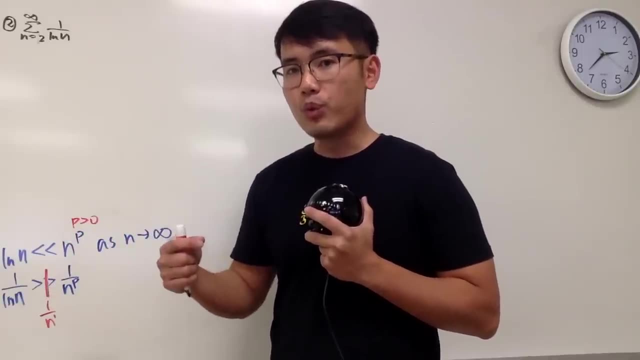 somewhere right here, when p is equal to 1.. Well, remember the p series. if p is greater than 1,, then that series converges. If p is less than or equal to 1, then that series diverges. If p: 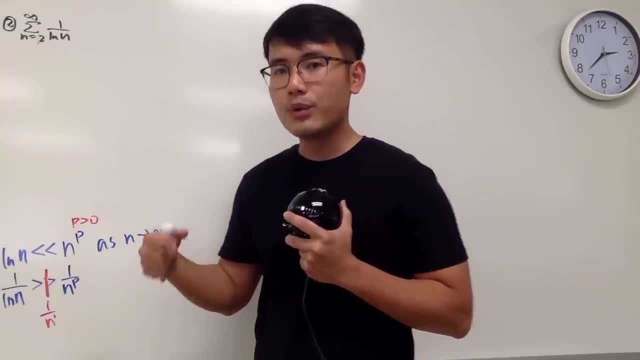 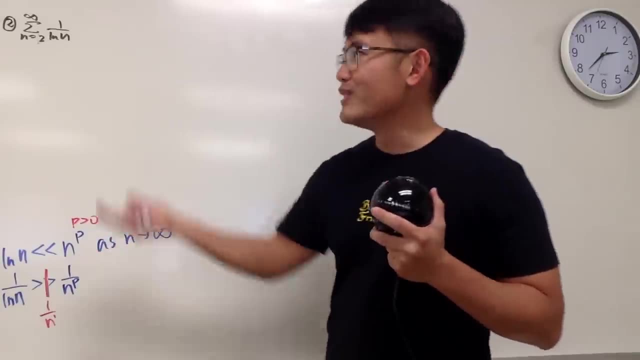 is greater than 1, it converges, And if p is less than or equal to 1, the series diverges. Okay, And then you can see that this is bigger than 1 over n. So of course, you can see that this right here. 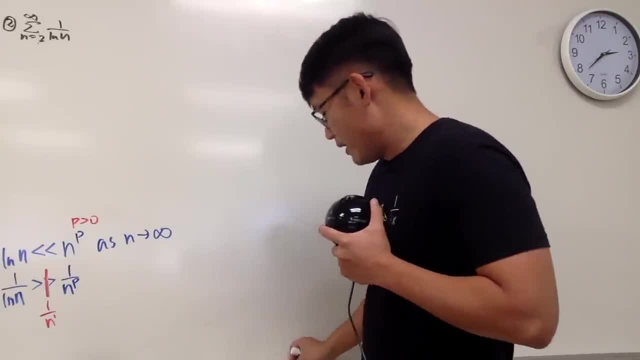 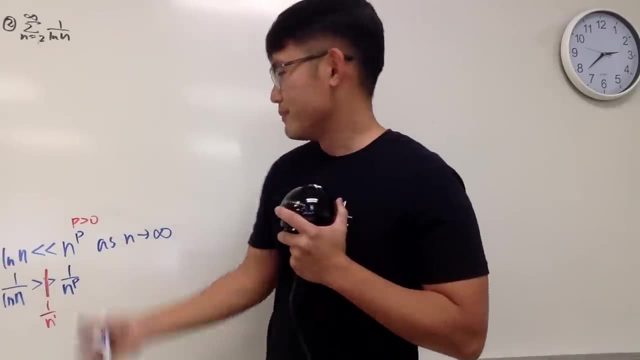 diverges by the least. So I will just show you guys how we can write this down the quicker way, right? So, and of course it also depends on your teacher, This right here is something that I allow my students to just use, and I think it's good. 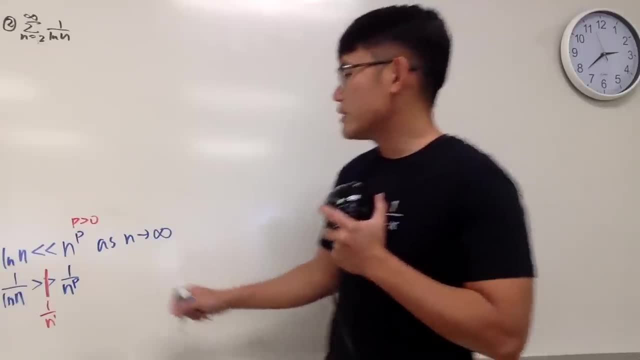 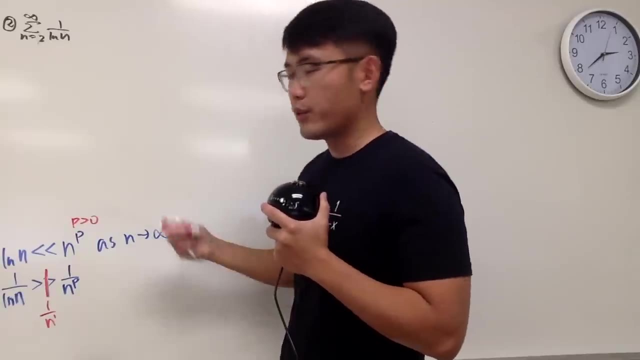 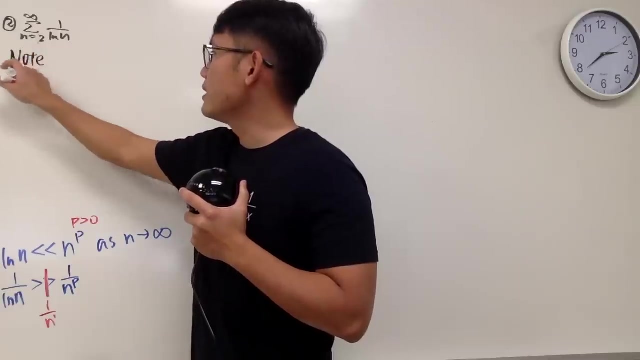 because they can compare the different kinds of infinity and all that. So the idea is that notice I'll just put down. this is how I will show work for you guys, right? So I will just say: note, Notice up to you, however you want to say it. 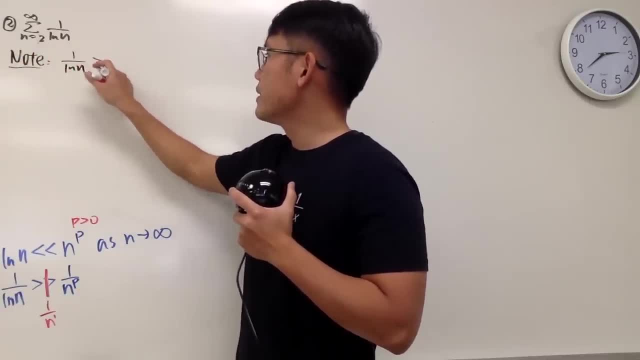 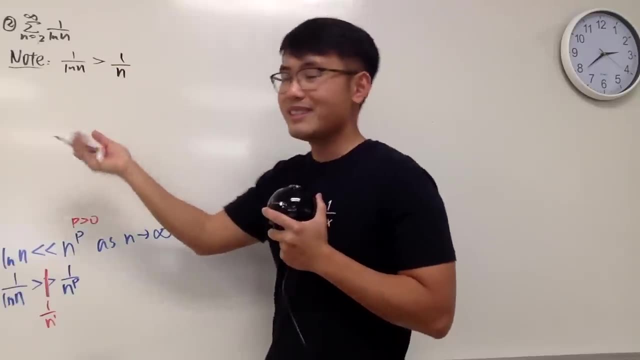 Note: 1 over ln, n is bigger than, but technically you don't have to put an equal sign because it's not equal anyway. 1 over n to the first power, like this For n greater than or equal to 2, because we are going from 2 to: 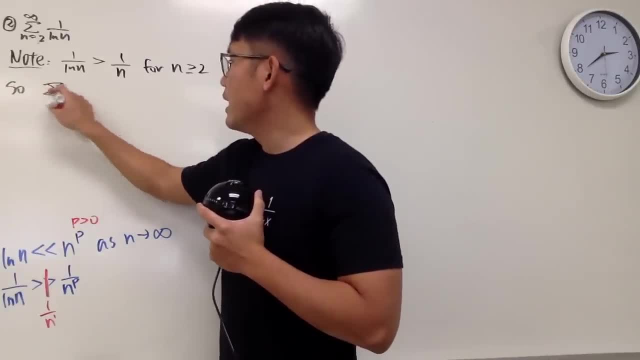 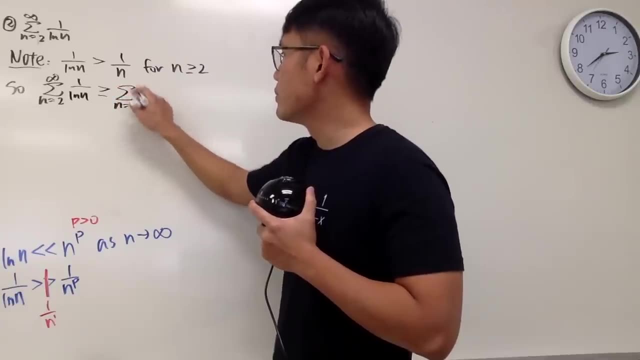 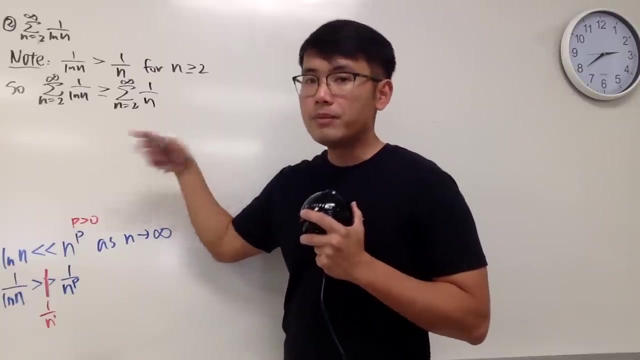 infinity. So the sum, as n goes from 2 to infinity, of 1 over ln, n is greater than or equal to the sum as n goes from 2 to infinity of 1 over n. like this. And now check this out Earlier the example: 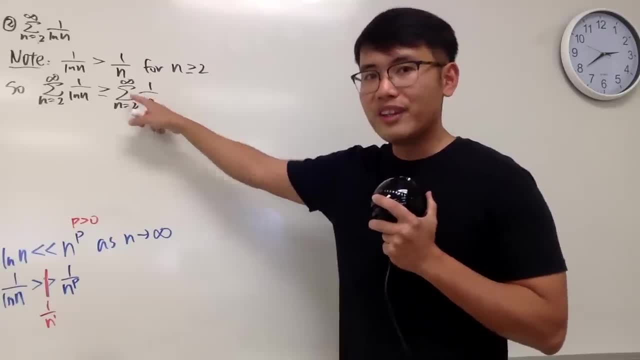 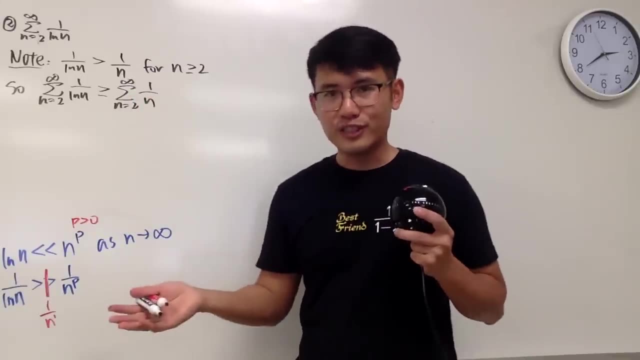 the question that we did was the sum, as n goes from 1 to infinity, of 1 over n to the first power, it diverges. But if you are going from 2 to infinity, that also diverges as well. The truth is the starting value right here, doesn't? 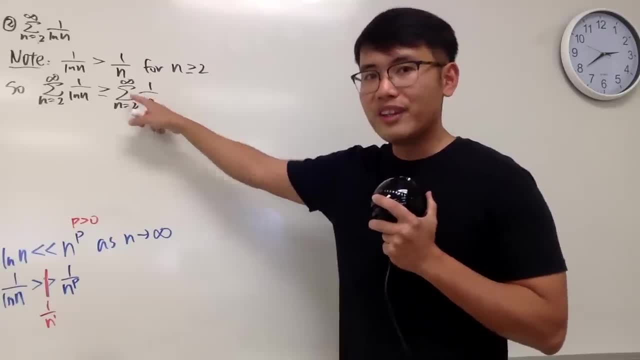 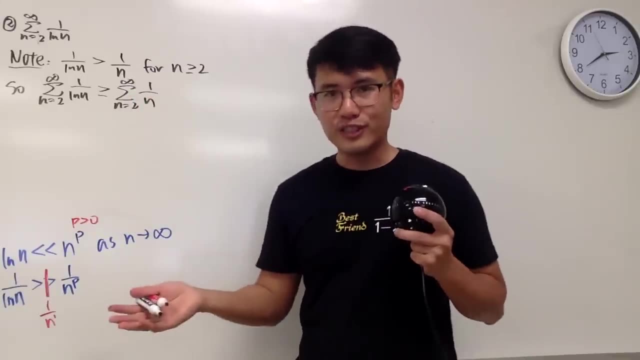 the question that we did was the sum, as n goes from 1 to infinity, of 1 over n to the first power, it diverges. But if you are going from 2 to infinity, that also diverges as well. The truth is the starting value right here, doesn't? 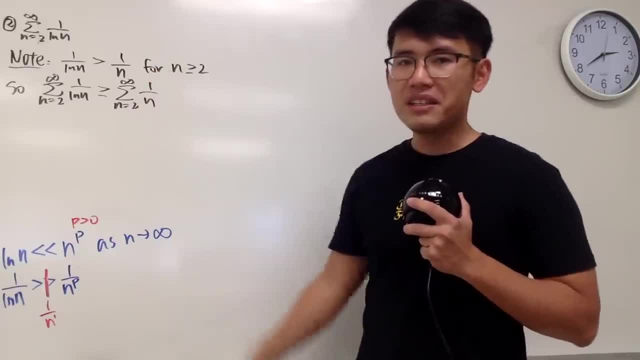 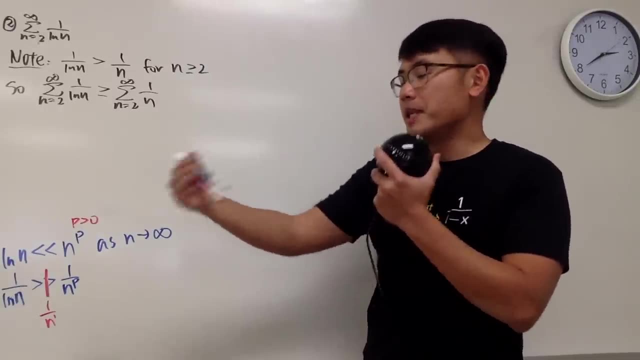 matter You can have. n is equal to 17 to infinity. This right here still diverges, Because you can ignore however many parts, however many terms in the front, that's just going to be finite anyway. It's the infinity part that you have to be worried about. 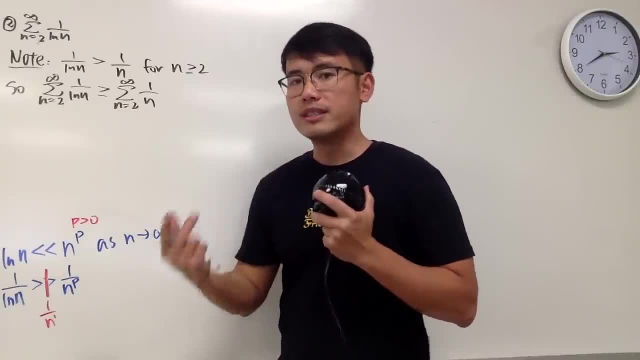 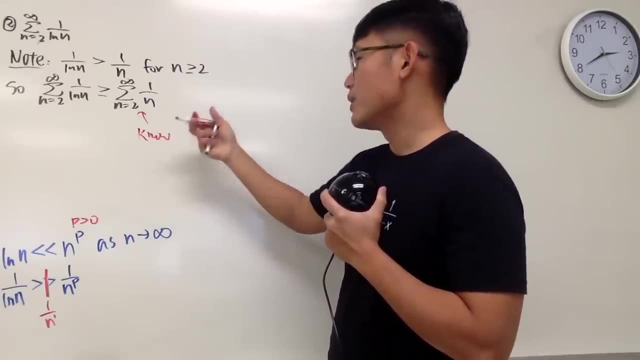 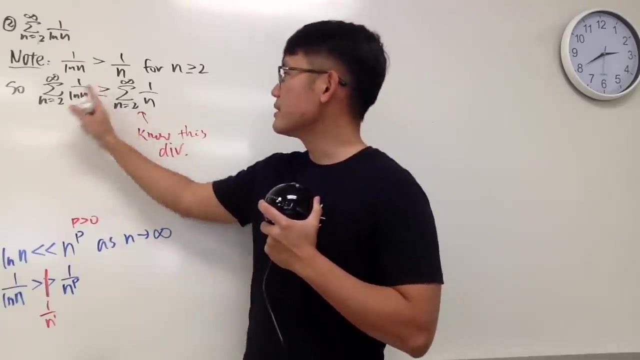 So, as you can see, this is the inequality that we can set up and we know this right here, we know well, we know this diverges and because this is bigger than that, we can say that this right here. 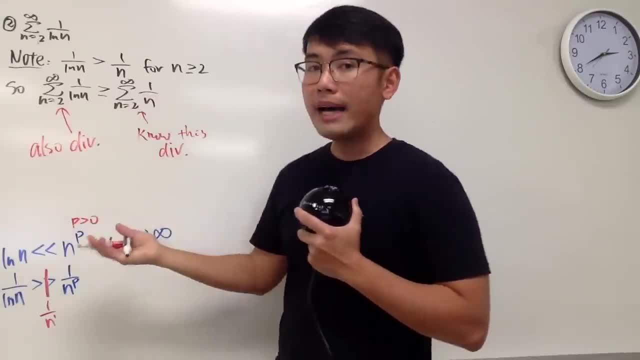 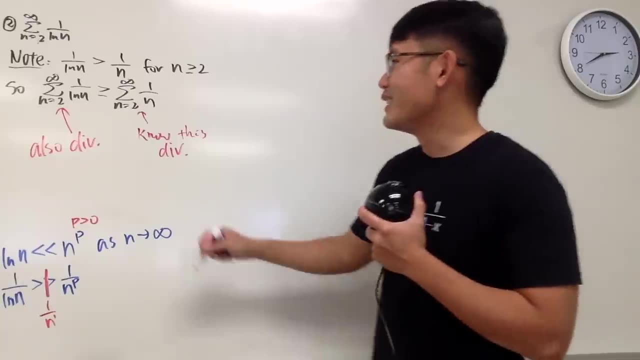 also diverges. Why? Because when you are bigger than an infinity, of course you have to be bigger than a. you have to be even bigger than infinity, right? It's like Thanos, Infinity stones, all that Alright, and 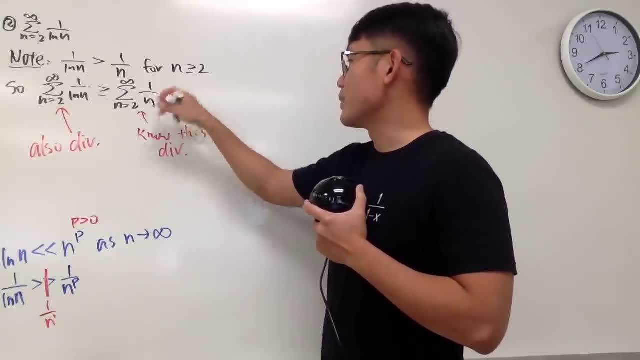 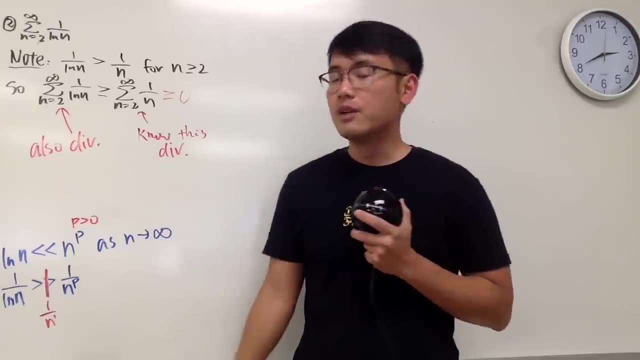 depends if you want to like indicate the zeros or not, Because when we are talking about the direct comparison test, we should also put this down, because both of them are positive right here. So be sure you put that down right. So. 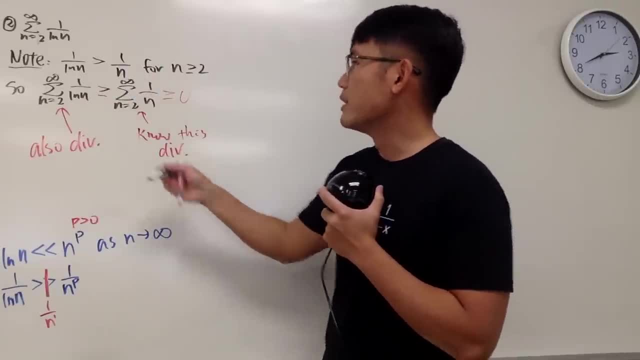 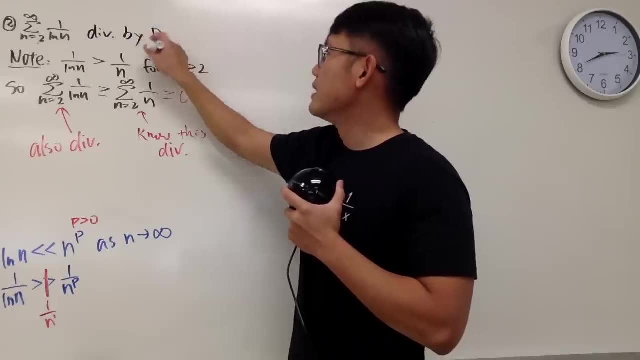 the conclusion that this right here diverges because of this right here. So I will just tell you guys, this right here Diverges. I will just put down by the direct comparison test, like that. So I will just put this: 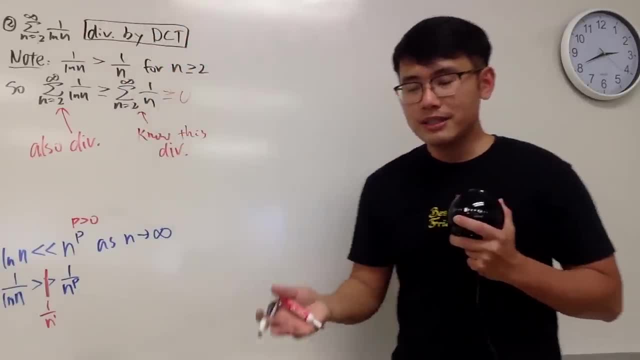 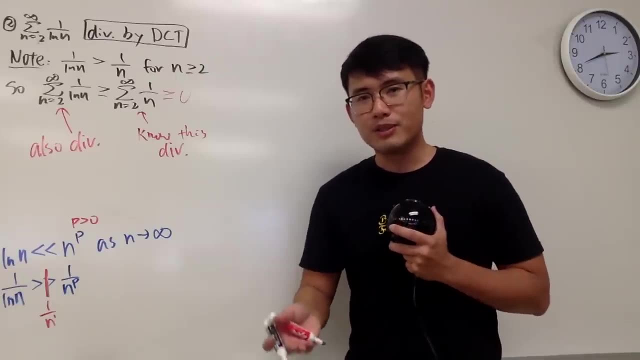 down for the answer, for simplicity purpose, And the truth is I was doing another video earlier, I was doing this one, but I was doing too much work and I realized I gave too much explanation. so ten questions took me like an hour or something. 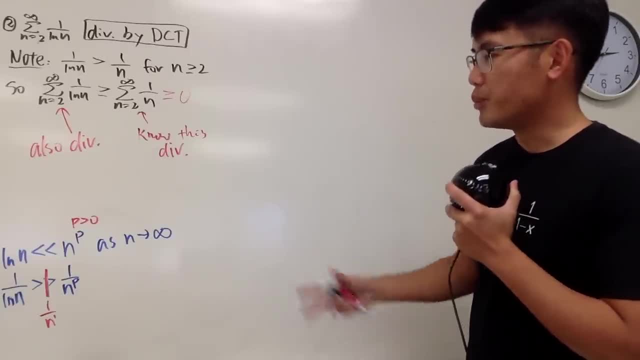 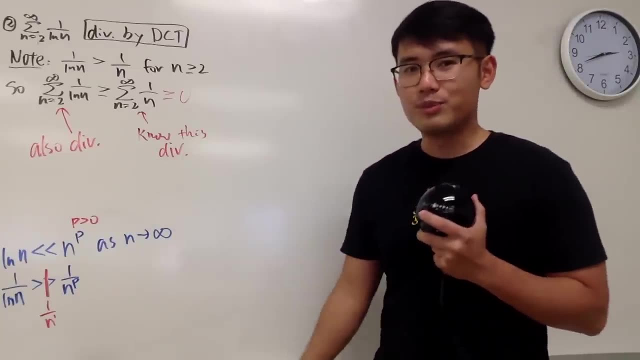 and I think that was not possible. so I would just like to give you guys the brief version of that, and I think this is still pretty clear and if you just write this down, you should still. you know your work is still pretty legit. 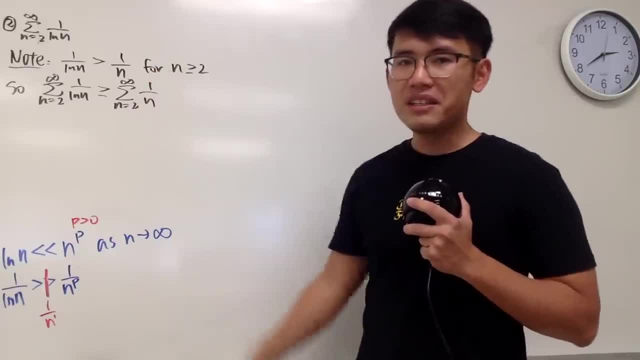 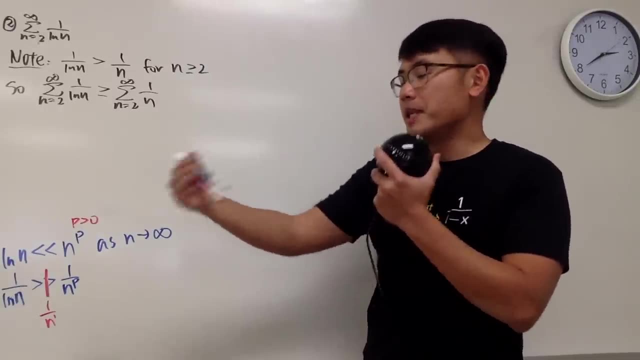 matter You can have. n is equal to 17 to infinity. This right here still diverges, Because you can ignore however many parts, However many terms in the front, That's just going to be finite anyway. It's the infinity part that you have to be worried about. 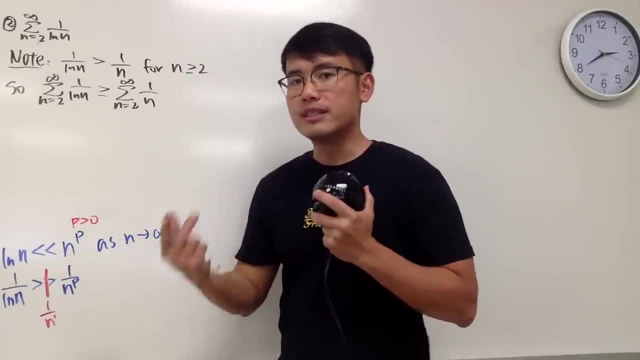 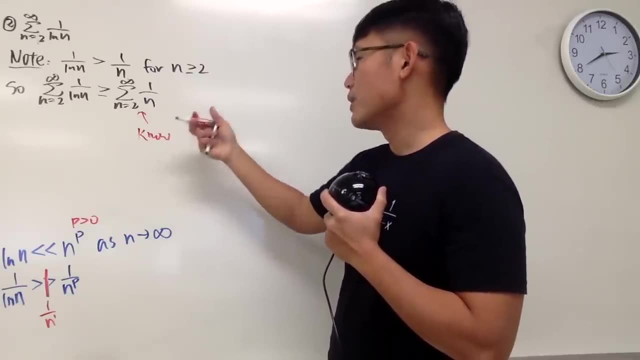 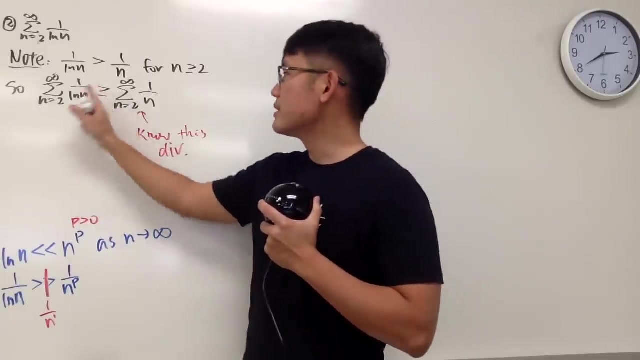 So, as you can see, this is the inequality that we can set up, And we know this right here, we know well, we know this diverges And because this is bigger than that, we can say that this right here also diverges. 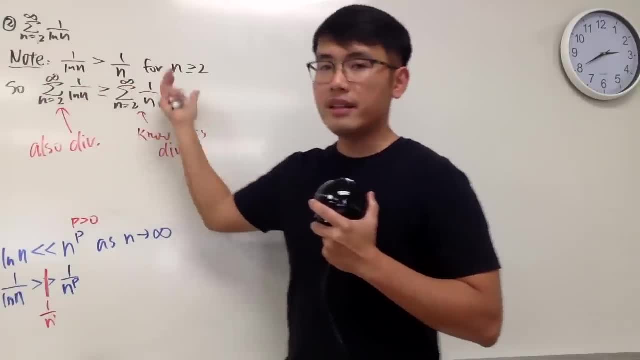 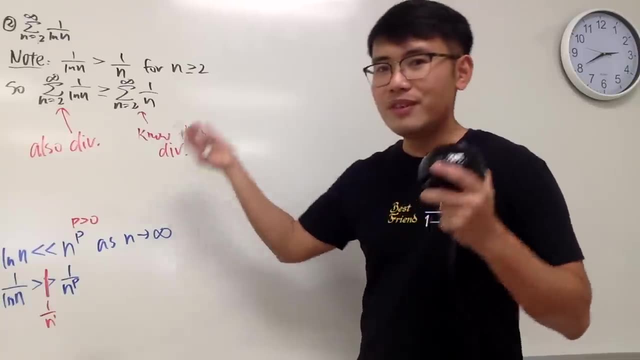 Why? Because when you are bigger than an infinity, of course you have to be bigger than a. you have to be even bigger than infinity, right? It's like Thanos, Infinity stones. all that, Alright, and depends, if you want to like, indicate the. 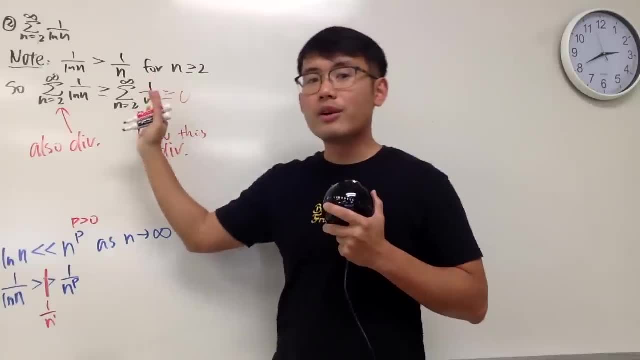 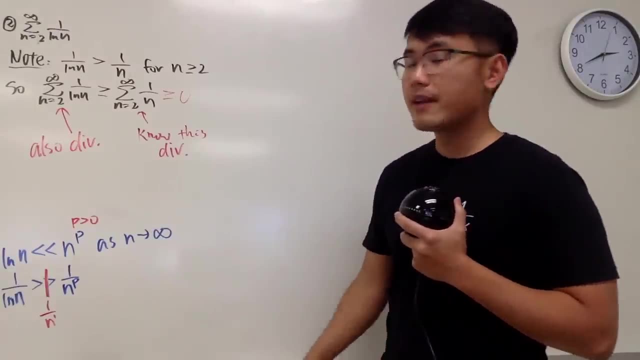 zeros or not, Because when we are talking about the direct comparison test, we should also put this down, because both of them are positive, right here. So be sure you put that down Right. So the conclusion that this right here diverges. 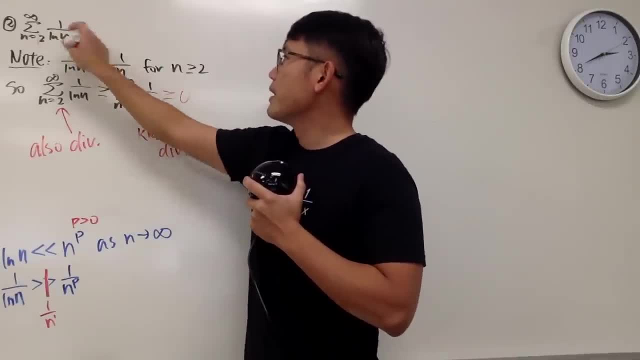 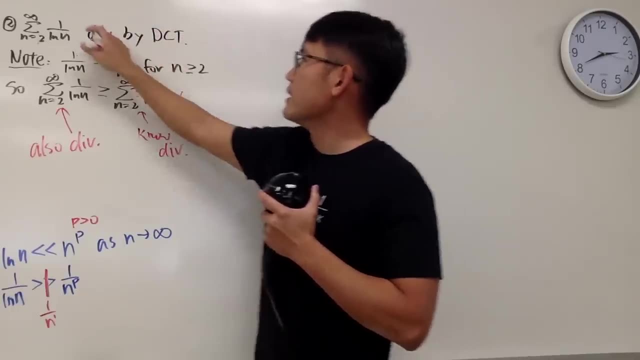 because of this right here. So we'll just tell you guys. this right here Diverges, I will just put down by the direct comparison test, Like that. So I will just put this down for the answer, for simplicity purpose. 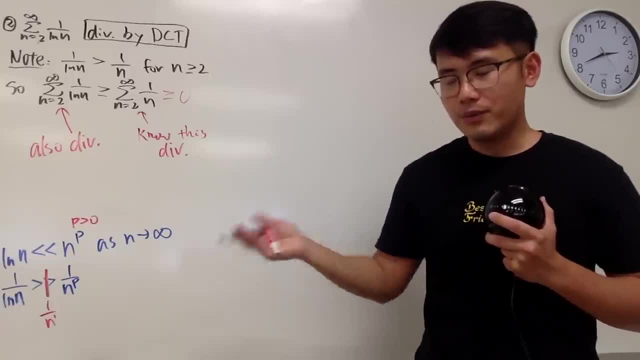 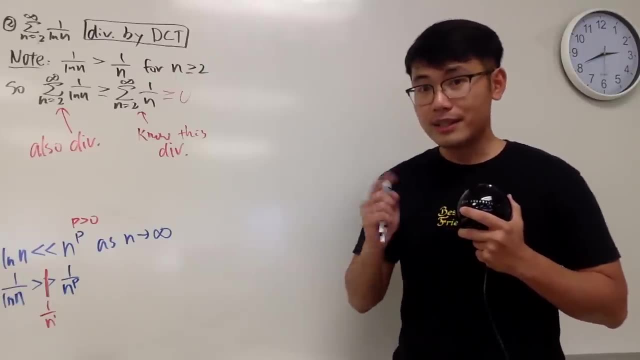 And the truth is I was doing another video earlier. I was doing this one, but I was showing too much work and I realized I gave too much explanation. so ten questions took me like an hour or something, and I think that was not possible. so I would. 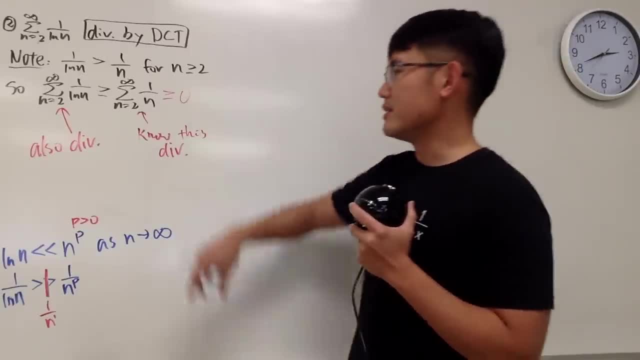 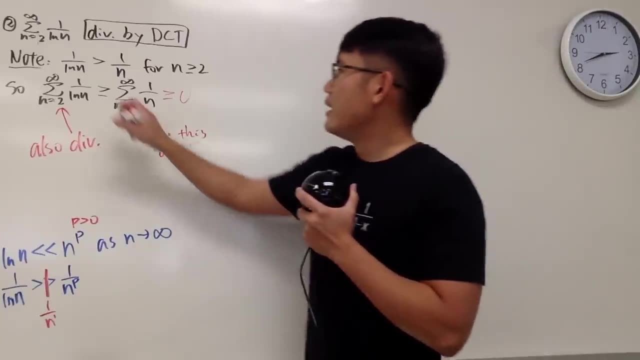 just like to give you guys the brief version of that, And I think this is still pretty clear and if you just write this down, you should still, you know your work is still pretty legit. Now this is, oh, I. 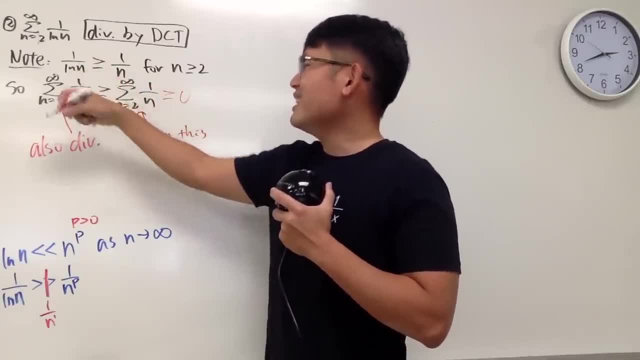 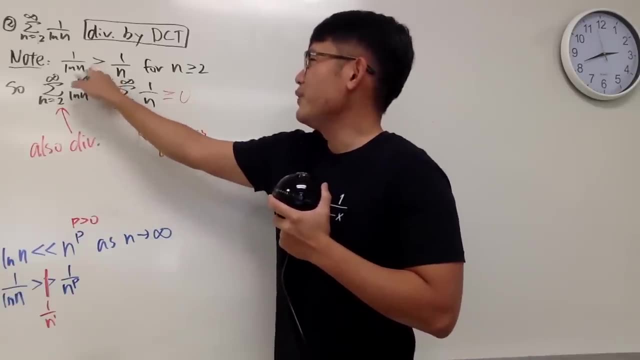 forgot to tell you: put on the equal sign. also Up to you. It's always you don't have the equal sign. Sometimes you put on equal sign, it doesn't matter. I forgot to say this is true and I forgot to tell you, guys, that. 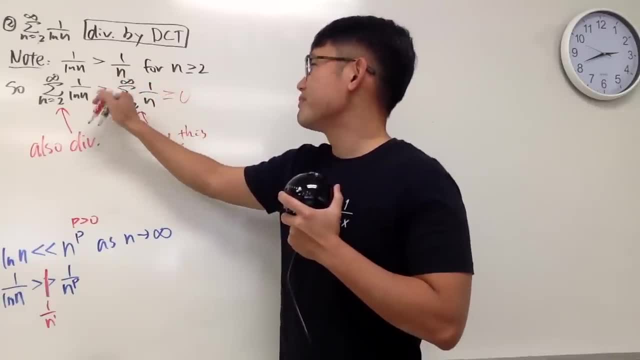 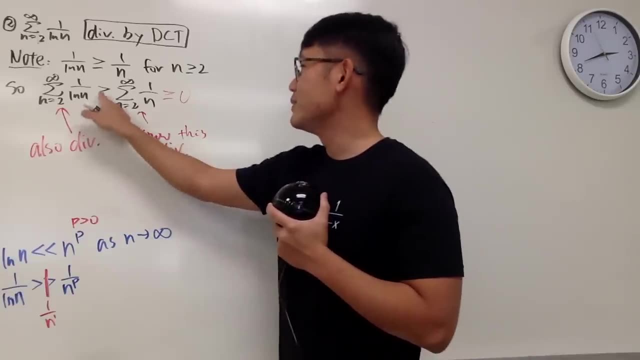 Now, this is well. I forgot to tell you: put on the equal sign. also Up to you. It's always you don't have the equal sign. Sometimes you put on equal sign, it doesn't matter. I forgot to say this is true. 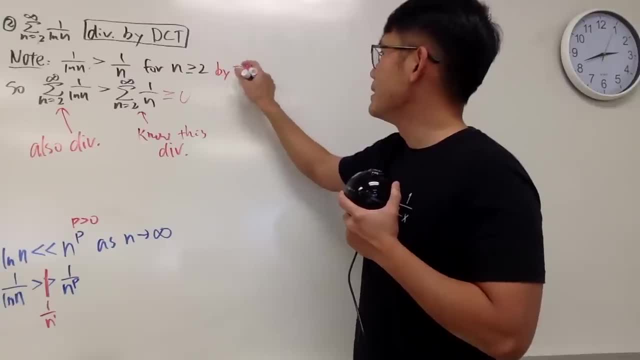 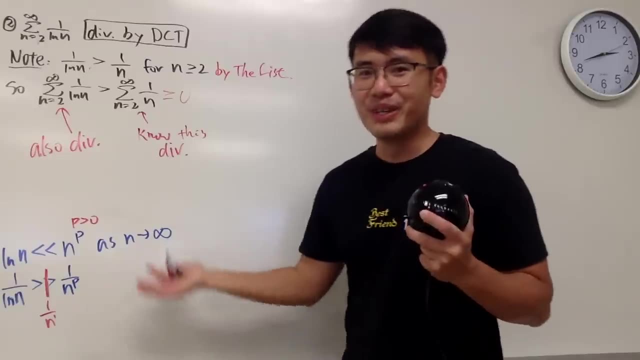 and I forgot to tell you guys that I have to tell you by the list, Right? So you have to give a reason. so if you give a reason by the list, then you are good to go. So that's the deal, Right? So 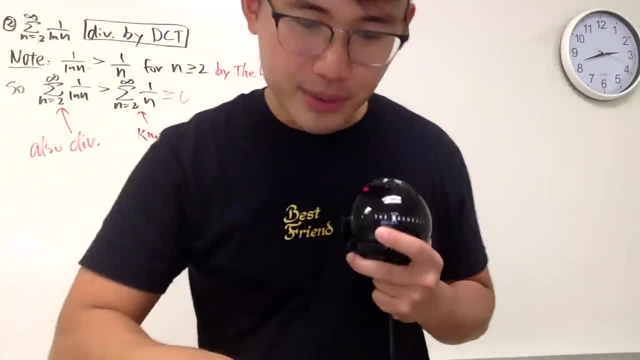 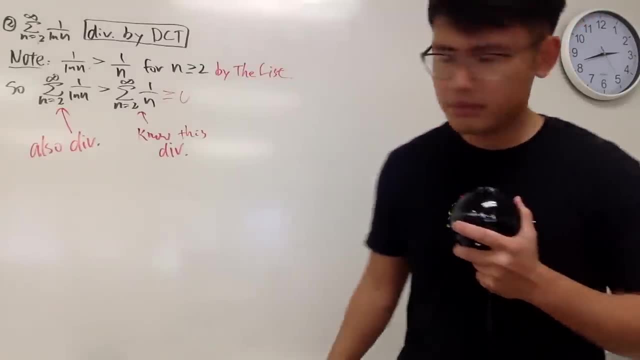 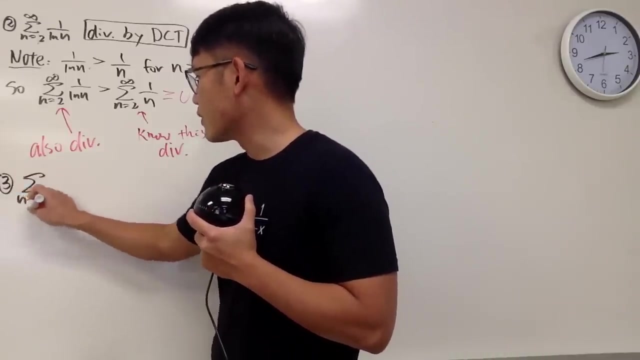 that's great. Now here we go. question number three: Oops, oh my god, We have natural log of n to the nth power. my god, Ah no, Let's see who did that. The sum as n goes from 2 to. 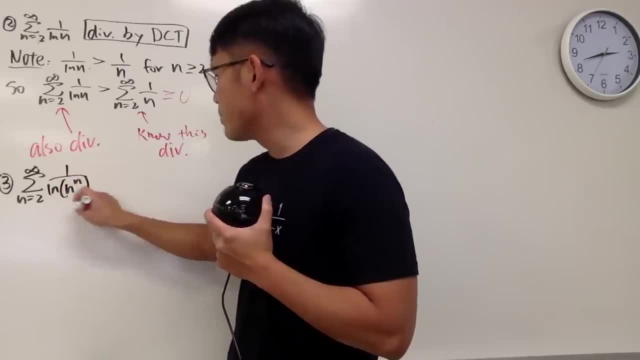 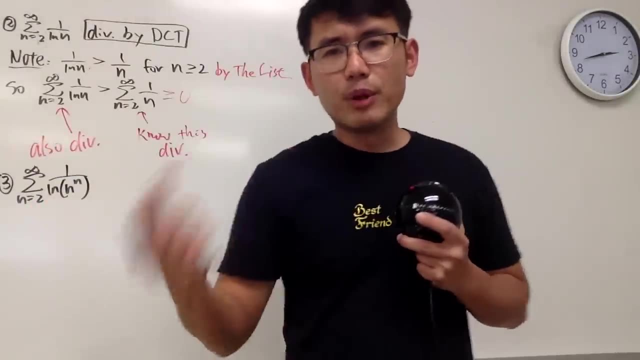 infinity 1 over natural log of n to the nth power. Well, as I told you, guys from the list ln, n is the smallest infinity, n to the n is the biggest infinity on the list, right When n goes to infinity. And now, 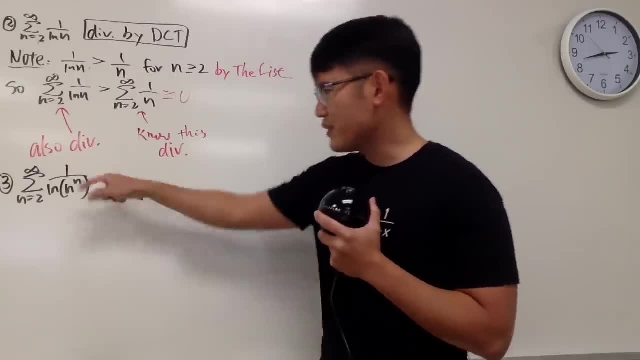 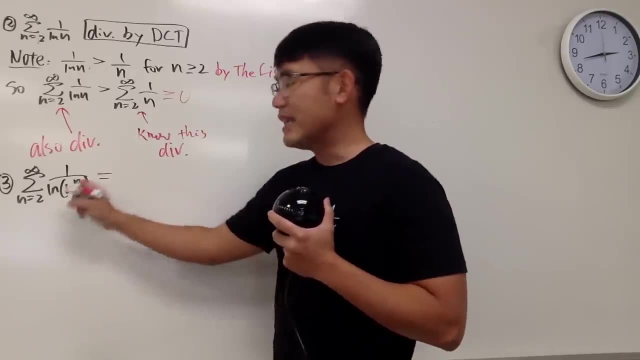 if you put n to the nth power instead of the ln, what happens? It looks scary, but it's actually not really, because, thanks to the natural log property, we can bring the power to the front. and this right here is just the sum as 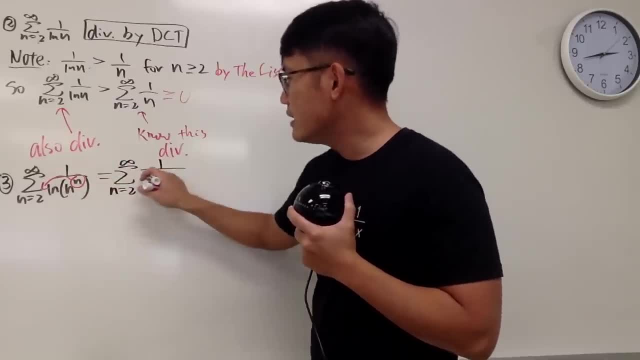 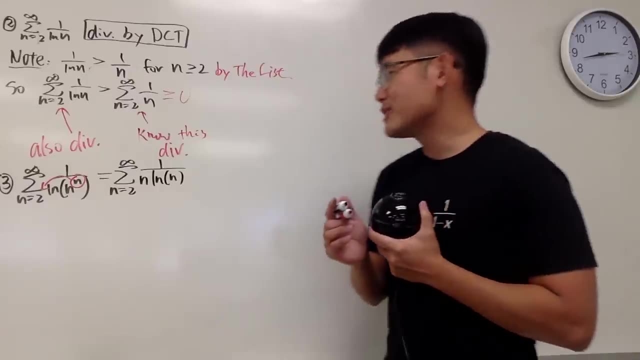 n goes from 2 to infinity, 1 over n times natural log of n like this. And now, what good does this do? Well, maybe we can do some kind of comparison, huh, But the problem is that, because this is, 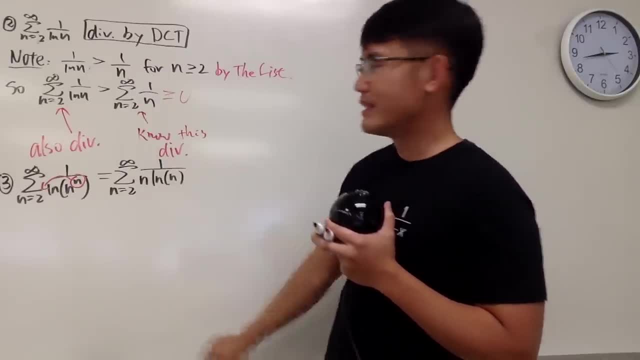 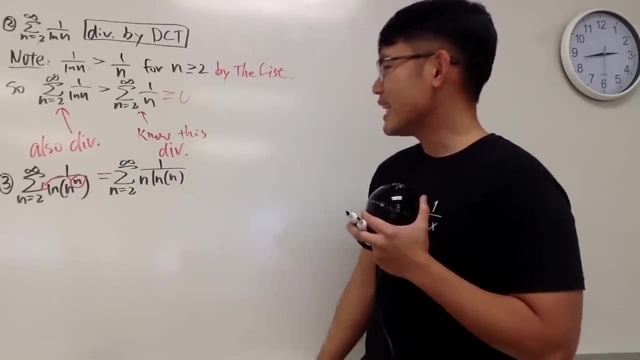 Okay, this diverges. This also diverges because that's question number one. this is question number two, right? The problem is that if you do this kind of inequality comparison, namely the direct comparison test, it's not going to. 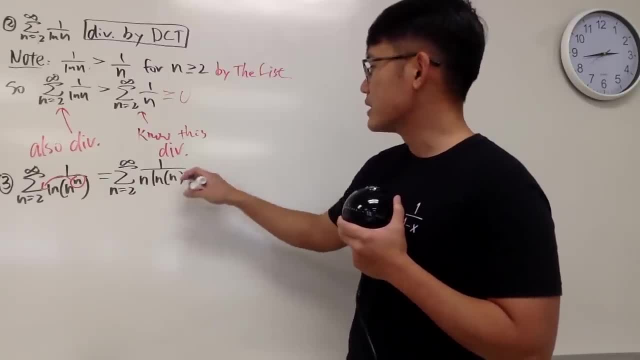 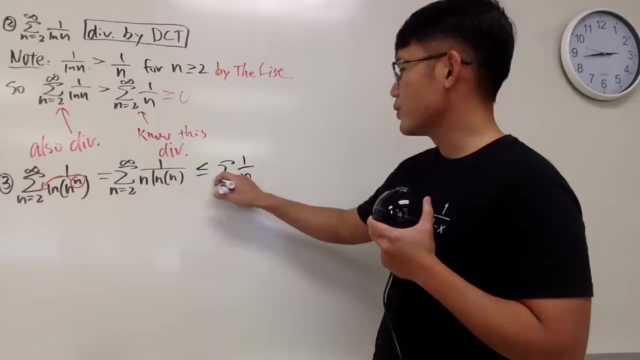 work out so well, because if you compare this with yes, this is less than or equal to. if you ignore that part, for example, the sum as 1 over as n goes from 2 to infinity, like this: This is true. 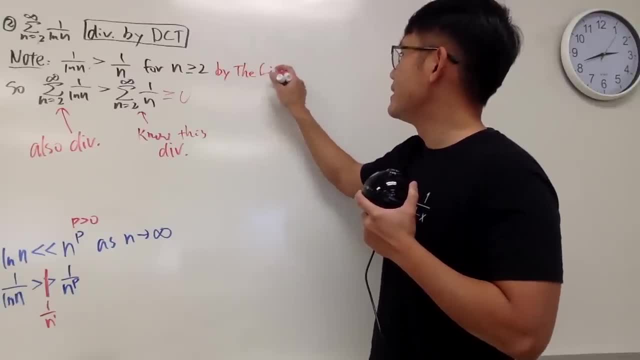 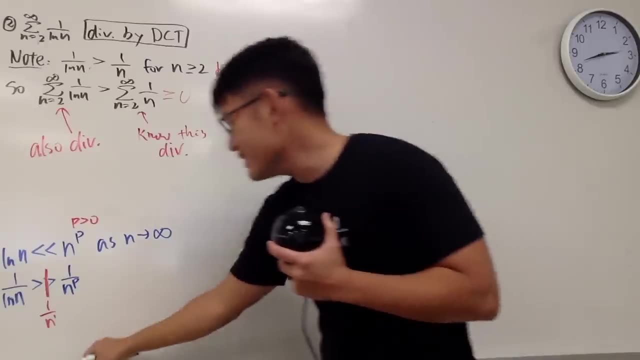 I want to tell you: by the list, Right. So you have to give a reason. so if you give a reason by the list, then you are good to go. So that's the deal, Right? So that's great. Now here we. 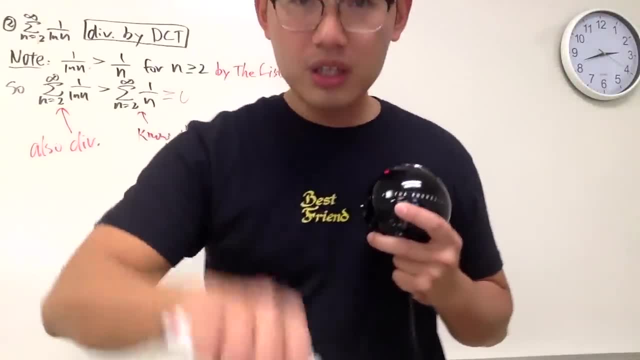 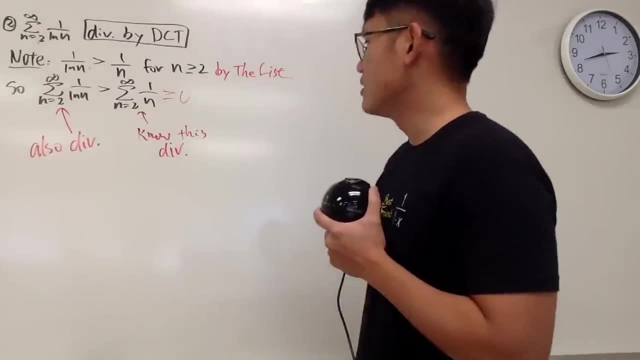 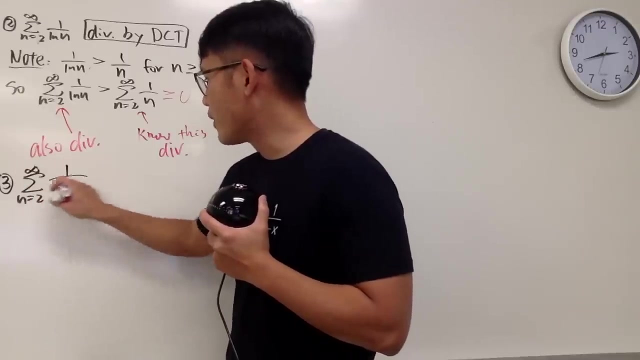 go. question number three: Oops, oh, my god, We have natural log of n to the nth power. my god, Oh no, Let's see who did that. The sum as n goes from 2 to infinity, 1 over natural. 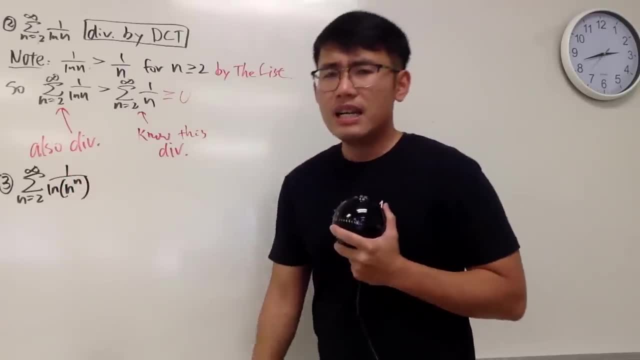 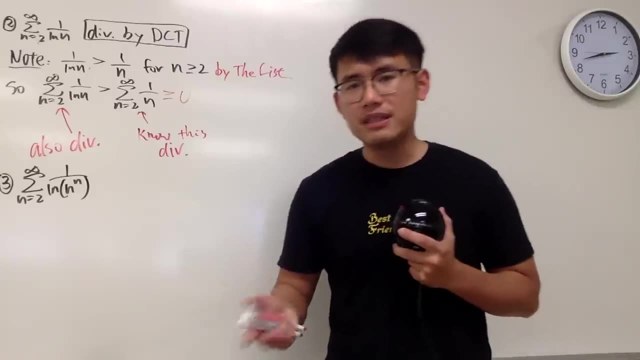 log of n to the nth power. Well, as I told you guys, from the list ln, n is the smallest infinity, n to the n is the biggest infinity on the list, right When n goes to infinity. And now, if you put n to the nth power, 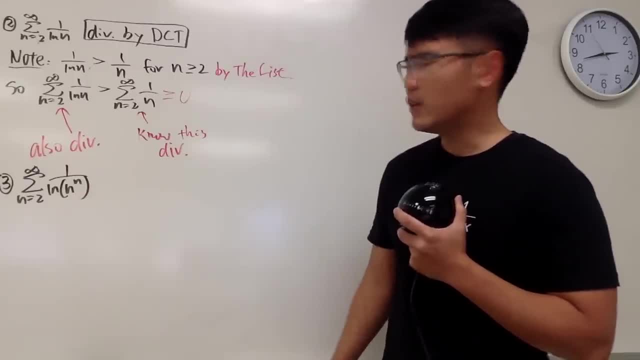 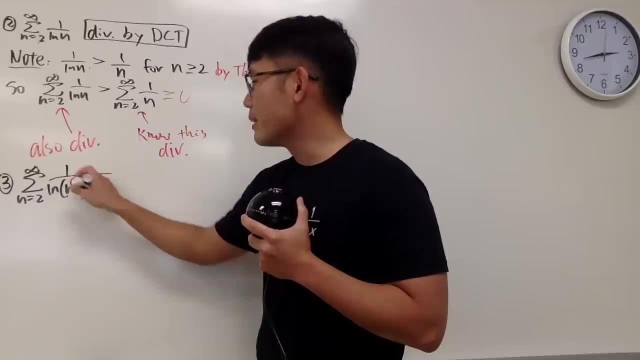 instead of the ln. what happens? It looks scary, but it's actually not really, because, thanks to the natural log property, we can bring the power to the front. and this right here is just the sum as n goes from 2 to infinity. 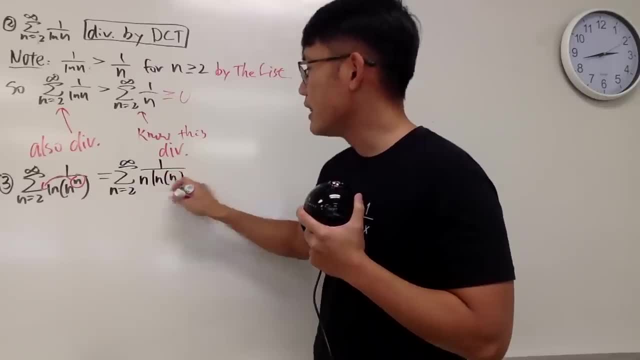 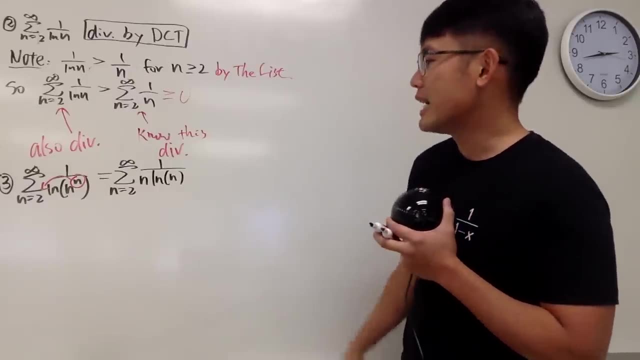 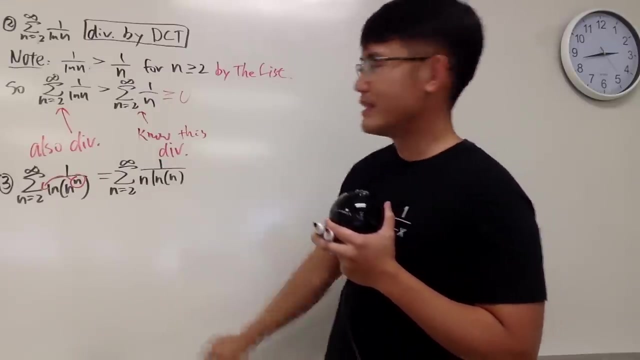 1 over n times natural log of n like this. And now, what good does this do? Well, maybe we can do some kind of comparison, huh, But the problem is that, because this is Okay, this diverges. This also diverges because 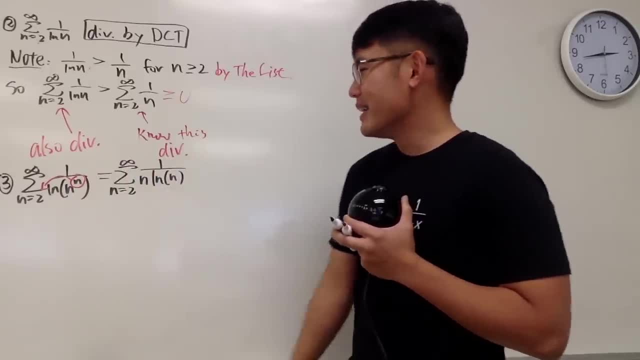 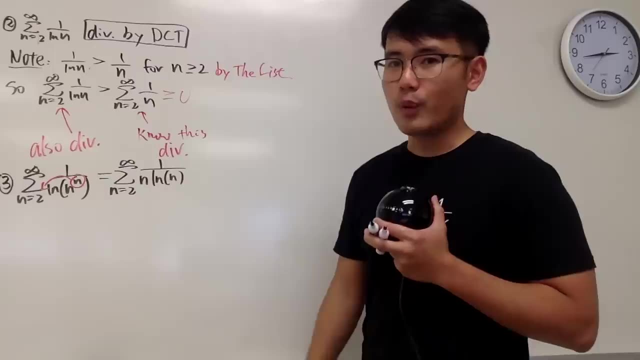 that's question number one. this is question number two, right? The problem is that if you do this kind of inequality comparison, namely the direct comparison test, it's not going to work out so well, Because if you compare this with yes, this is less than or equal to. 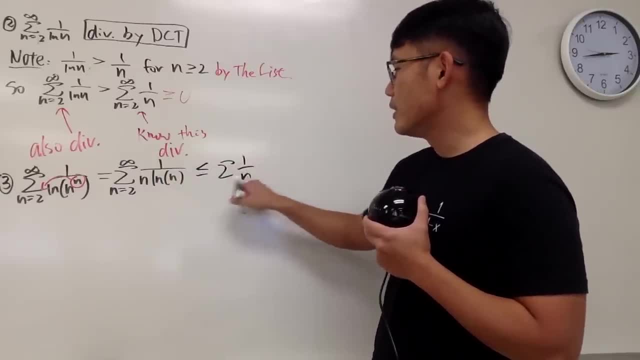 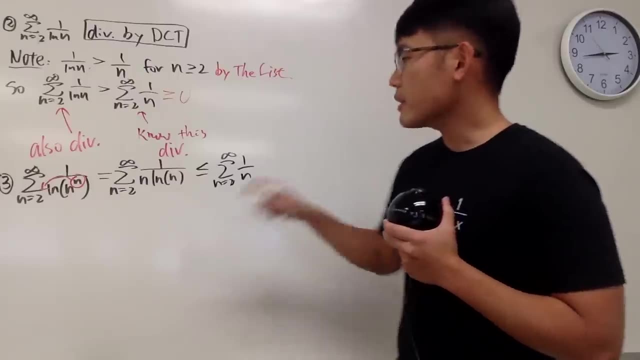 if you ignore that part, for example, the sum as 1 over as n goes from 2 to infinity, like this. This is true, right, This inequality is true. However, the problem is this diverges but when you have something. 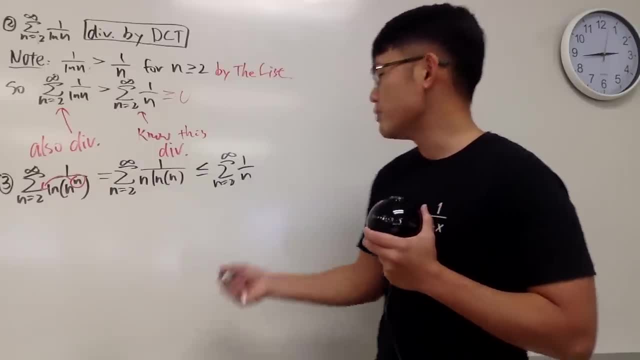 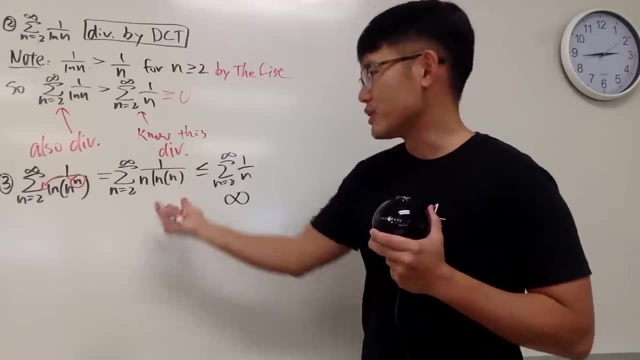 that's less than a divergent. you cannot draw a conclusion Because, remember, this right here is infinity, This right here it's. well, you don't know if it's a smaller version of infinity or it's just finite And the 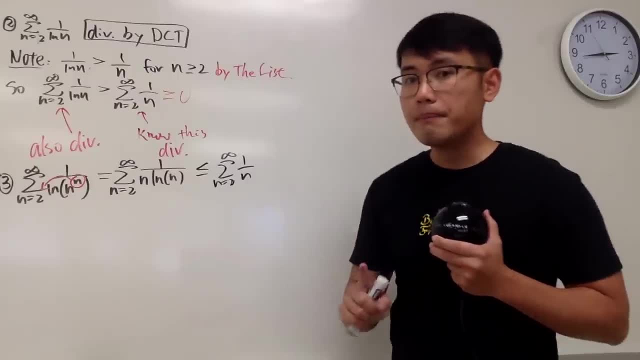 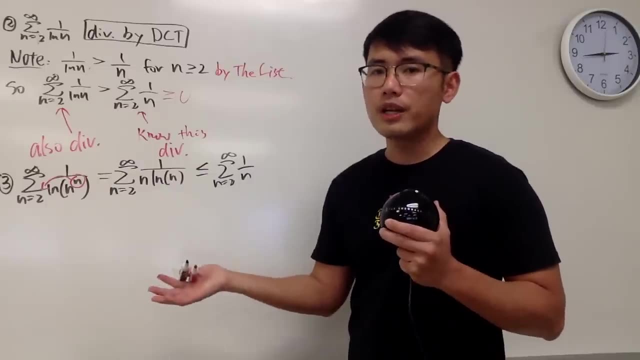 right, This inequality is true. However, the problem is this: diverges, but when you have something that's less than a divergent, you cannot draw a conclusion because, remember, this right here is infinity, this right here it's. well, you don't know if 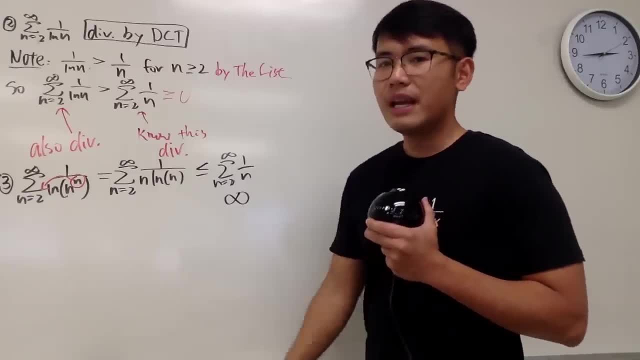 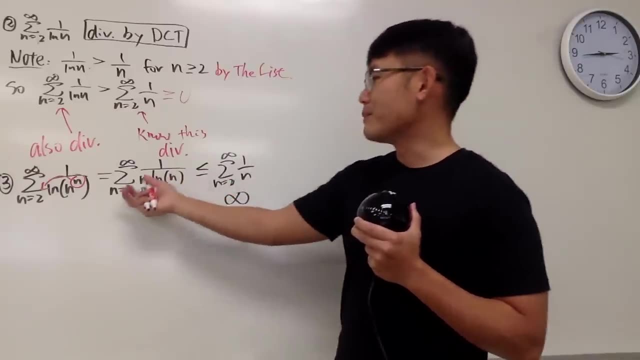 it's a smaller version of infinity or it's just finite, And the analogy I want to give my students is that imagine this is like a, like an older person, and if you have somebody who is younger than an older person, what can you say about this? 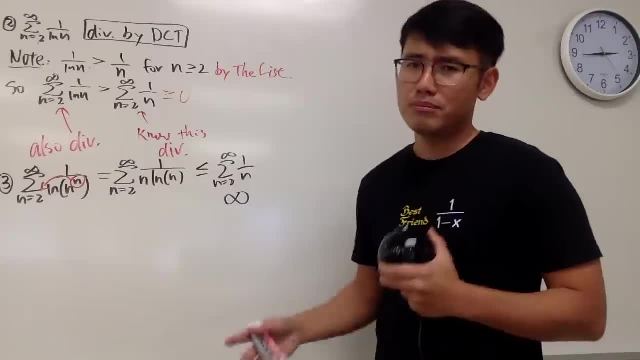 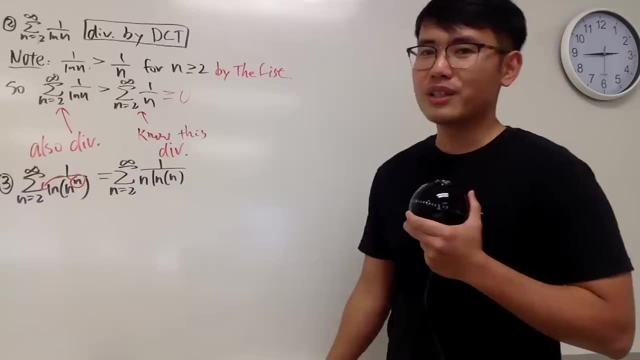 person. Is he old? No, Is he young? No, It depends. I don't know. yet We have to do more work on that right. So unfortunately, direct comparison test doesn't really work, Of course, if you put. 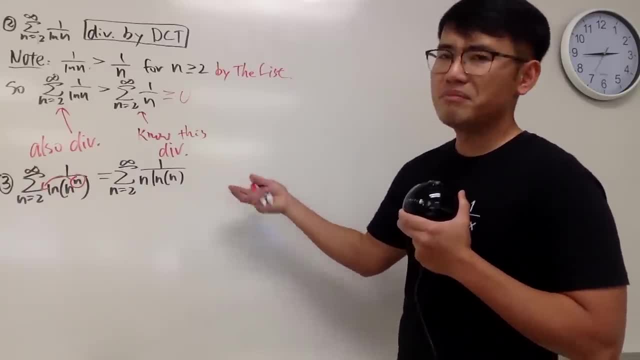 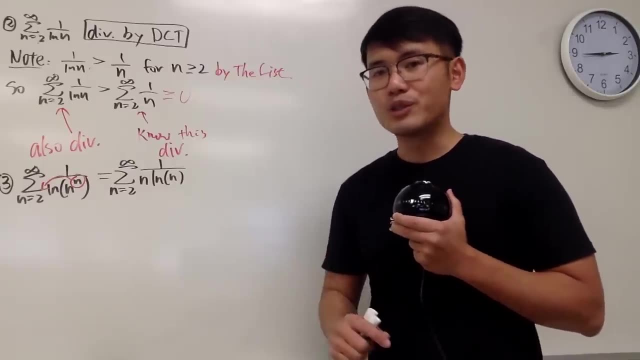 down the direct comparison test with 1 over natural log of n. again the inequality still doesn't work. You can try to do it with limit comparison test but unfortunately you'll get either 0 or infinity. It's tricky, But you know, I feel like doing some integral. 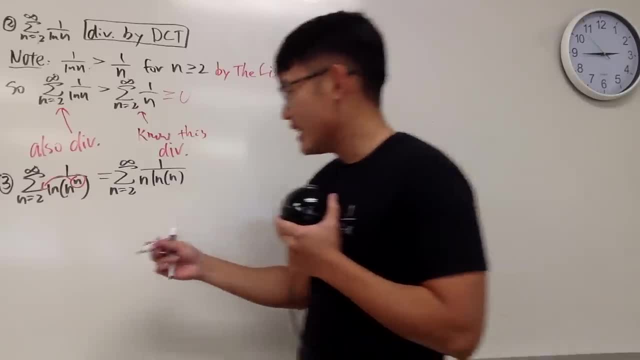 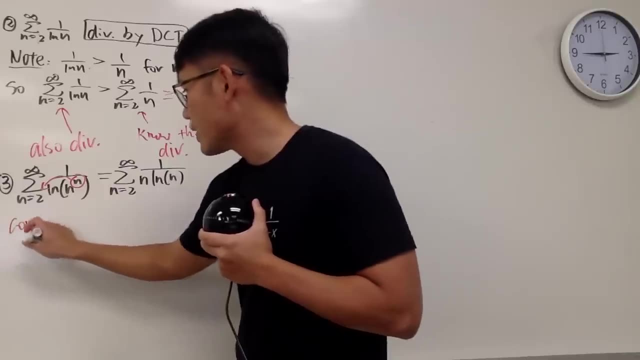 so we'll do some integral. So this is how we are going to do it, Because I notice 1 over x, ln x is something that we can actually integrate. So here we go. We are going to consider, and I will just take this: 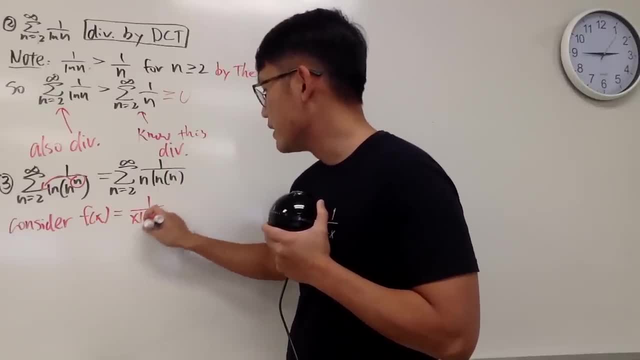 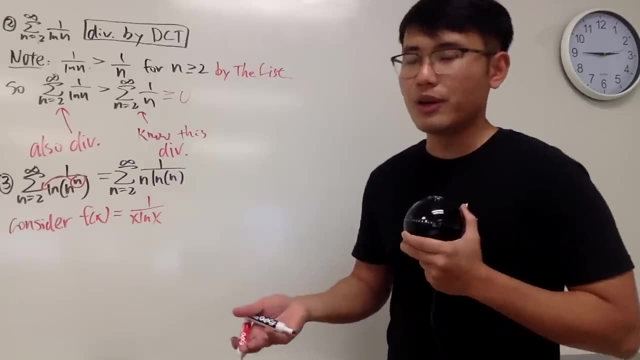 to be f of x as 1 over x, natural log of x. right here I will consider this function and notice. and again, it depends on your teacher on how much work you have to show. But in order for us, 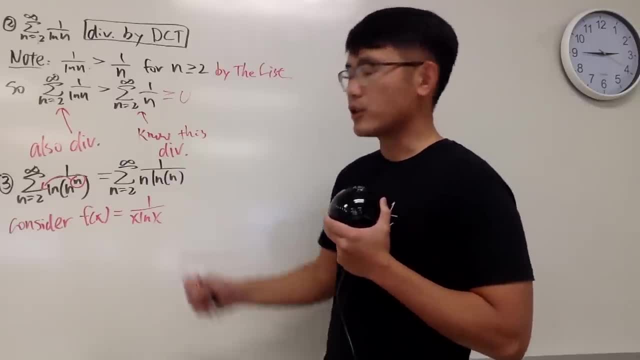 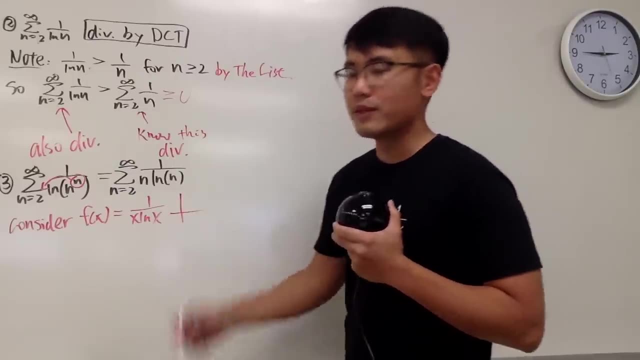 to use the integral test. we have to make sure this function is positive and it's also decreasing. So I will just suggest you guys at least to put a graph or something, and when n is 2, you can see that it's. 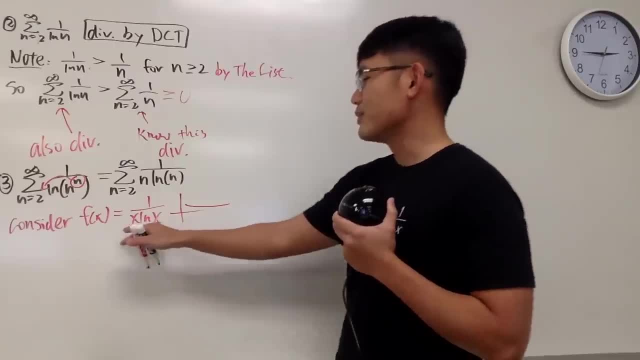 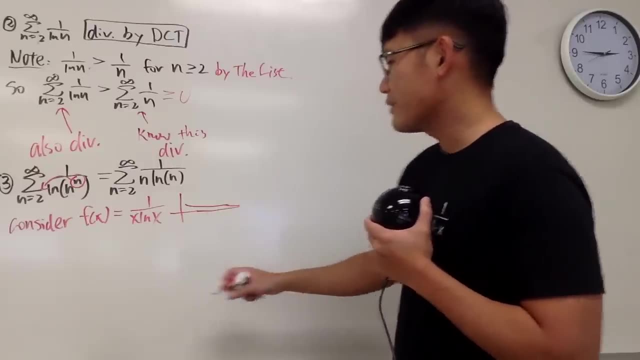 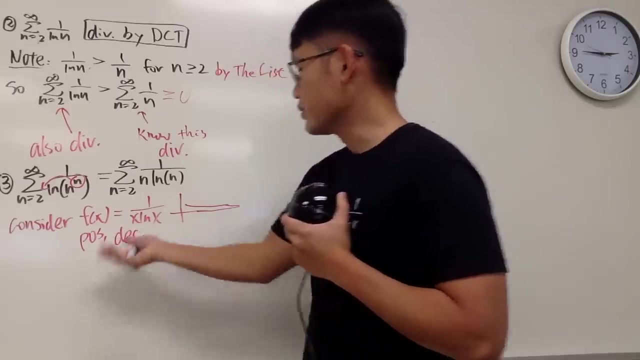 seriously. it's a decreasing function. As n goes to, as x goes to infinity, it approaches 0, so it's decreasing And it's always positive. So you can put a graph and you can say positive and decreasing. So just indicate. 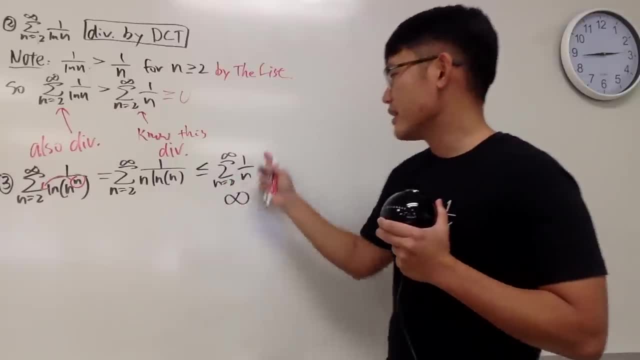 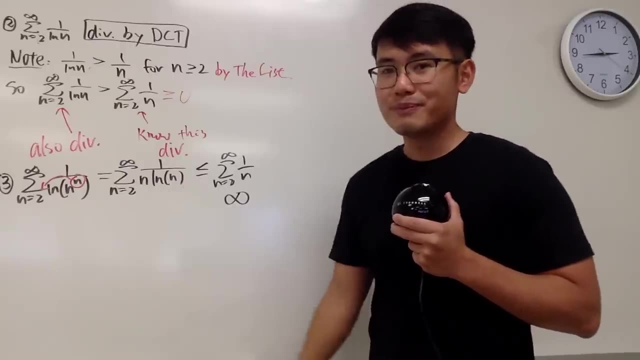 analogy I want to give my students is that: imagine. this is like a, like an older person, and if you have somebody who is younger than an older person, what can you say about this person? Is he old? No, Is he young- No? 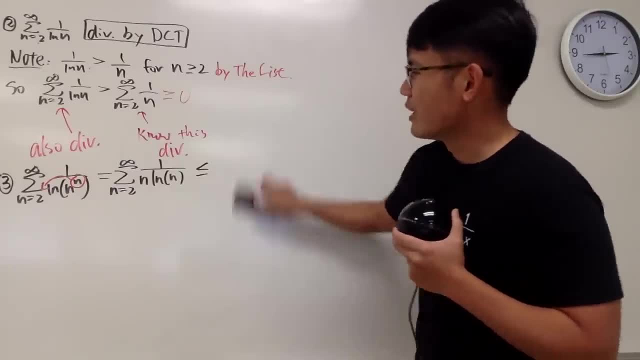 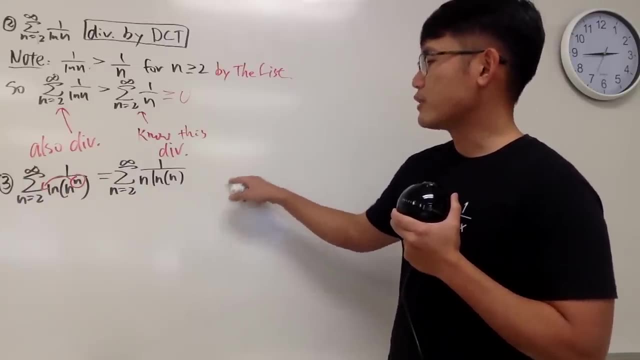 It depends. I don't know. yet We have to do more work on that right. So unfortunately direct comparison test doesn't really work. Of course, if you put down the direct comparison test with 1 over natural log of n again, 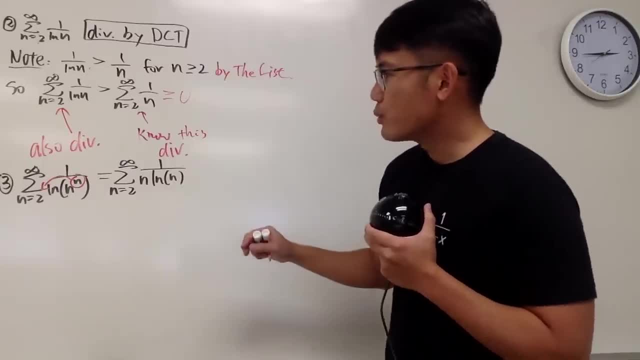 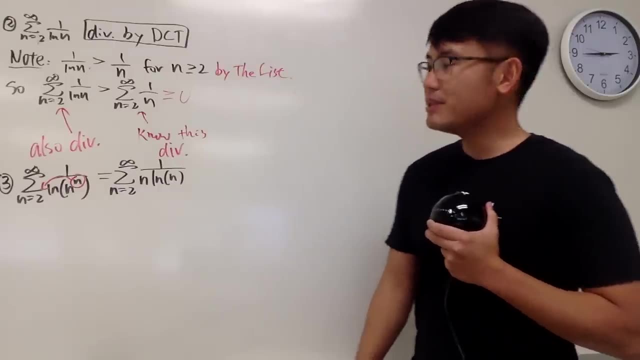 the inequality still doesn't work. You can try to do it with limit comparison test, but unfortunately you'll get either 0 or infinity. It's tricky, But you know, I feel like doing some integral, so we'll do some integral. So this is how. 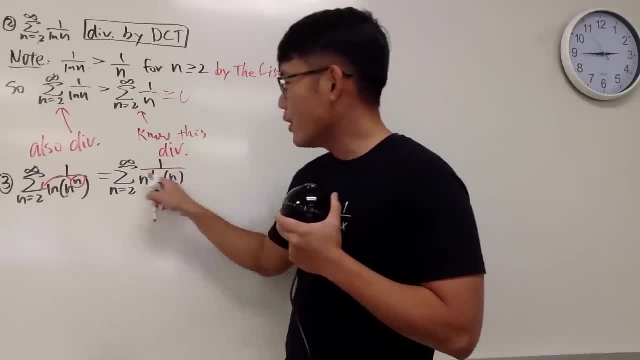 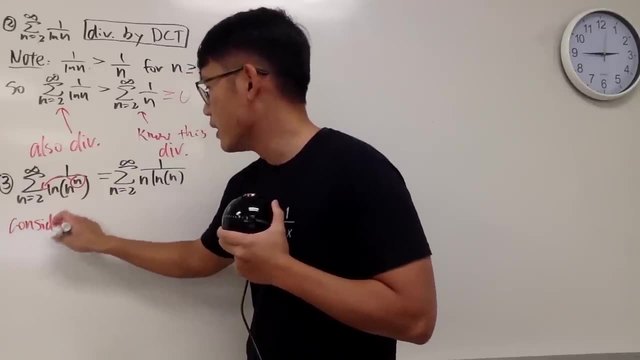 we are going to do it Because I notice 1 over x ln is something that we can actually integrate. So here we go. We are going to consider- and I will just take this to be f as 1 over x natural log. 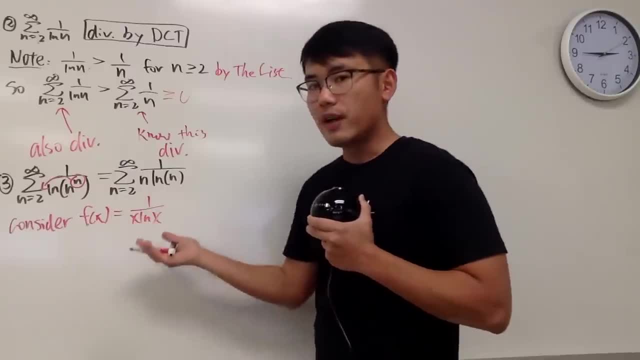 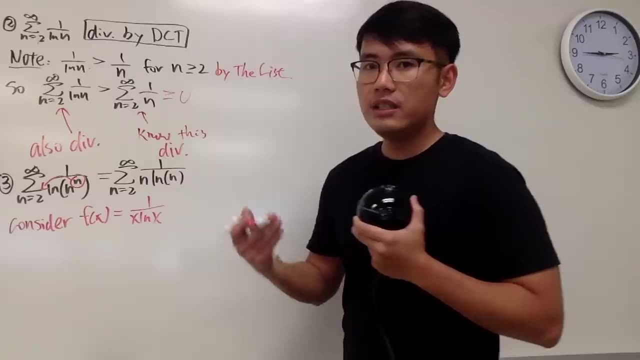 of x right here. I will consider this function and notice. and again, it depends on your teacher, on how much work you have to show. But in order for us to use the integral test, we have to make sure this function. 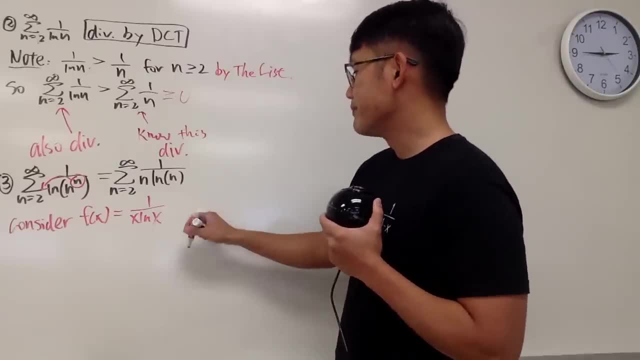 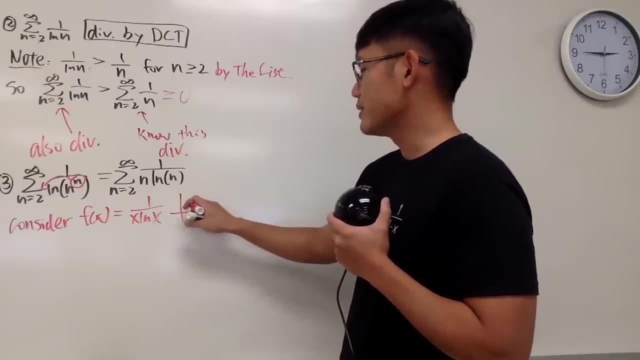 is positive and it's also decreasing. So I will just suggest you guys at least to put a graph or something. and when n is 2, you can see that it's seriously. it's a decreasing function. As x goes to infinity, it approaches. 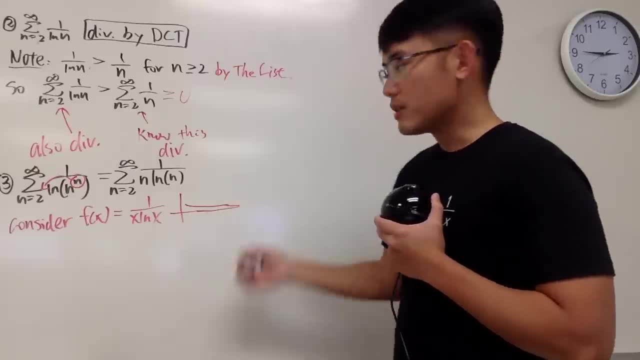 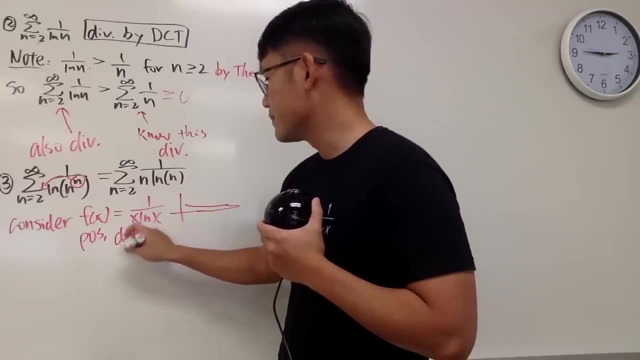 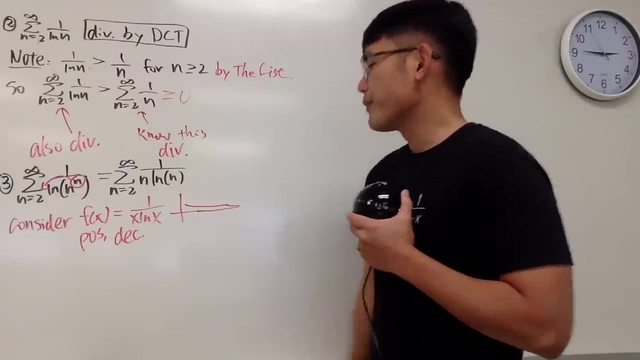 0, so it's decreasing, And it's always positive. So you can put a graph and you can say positive and decreasing. So just indicate that DEC stands for decreasing, not December. okay, We are not there yet, Alright, so 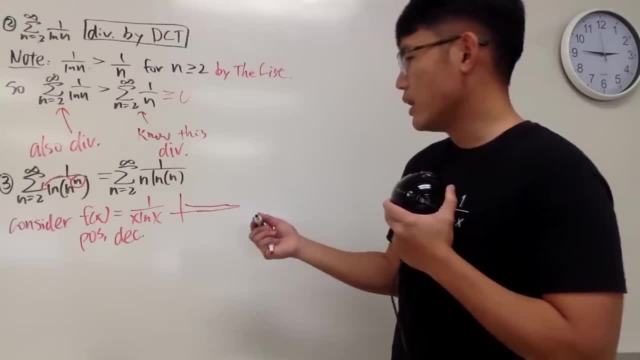 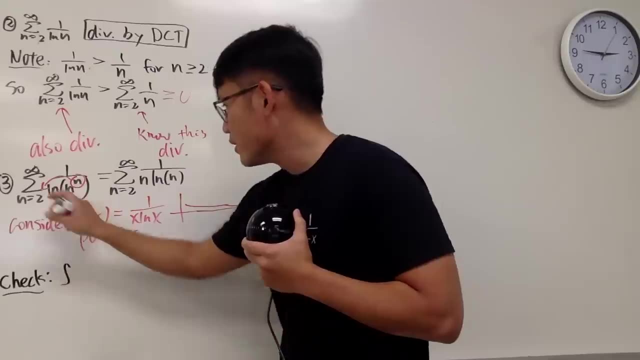 we are ready to go Now. this is the check that we will have to do. Let me just put it down right here. I think we should have enough space. Here we go integral time integrating from 2 to infinity, and we are going to just integrate. 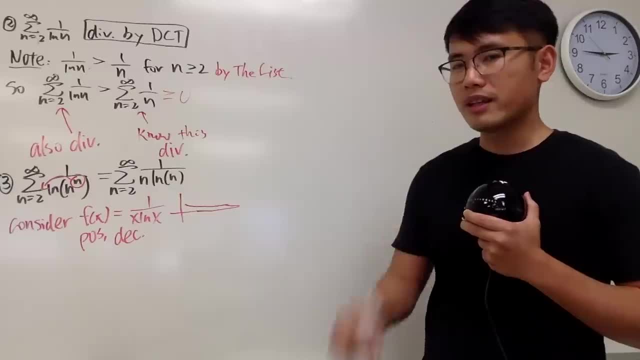 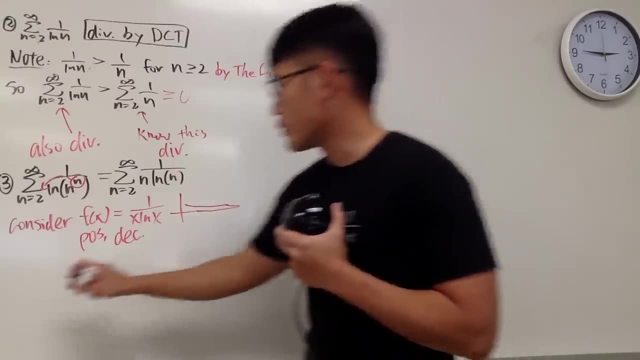 that DEC stands for decreasing, not December. okay, we are not there yet. Alright, so we are ready to go Now. this is the check that we will have to do. Let me just put it down right here. I think we should have enough space. 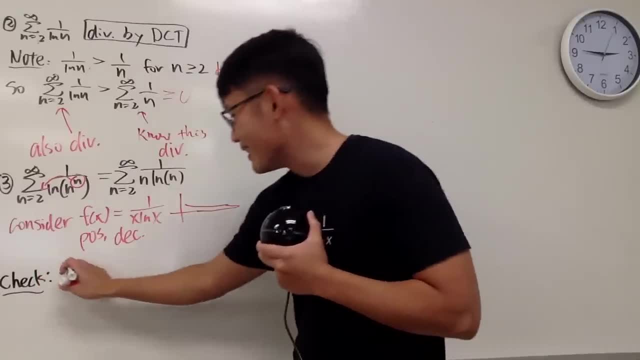 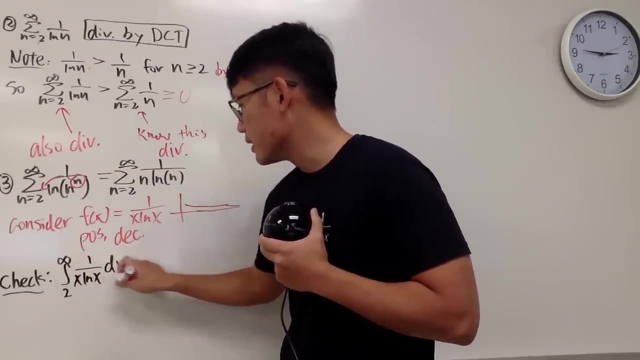 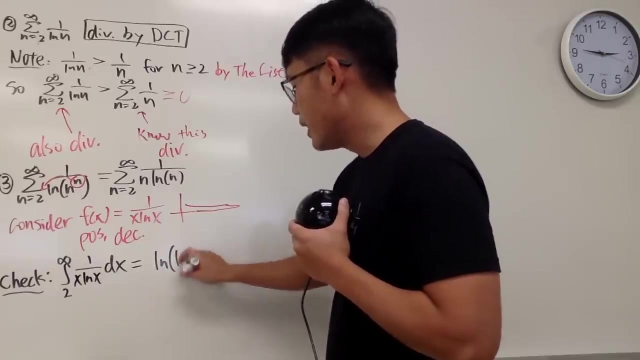 Here we go, Integral time, integrating from 2 to infinity, and we are going to just integrate 1 over x, ln, x, dx. Well, I will just tell you guys that when you integrate that, we get ln of ln x. Why? 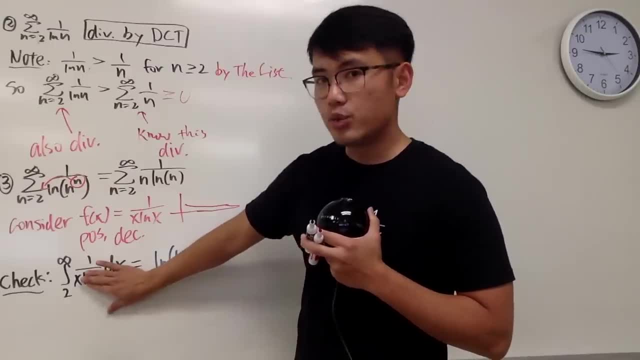 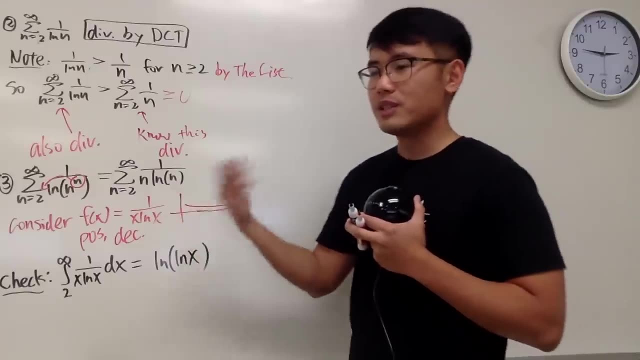 Because if you let u equal to ln x, the derivative of ln x is 1 over x, right? So if you just get it so that you end up with 1 over u and the integral of 1 over u is natural log of u. 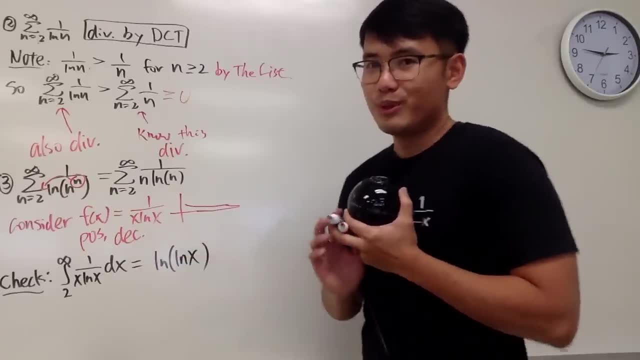 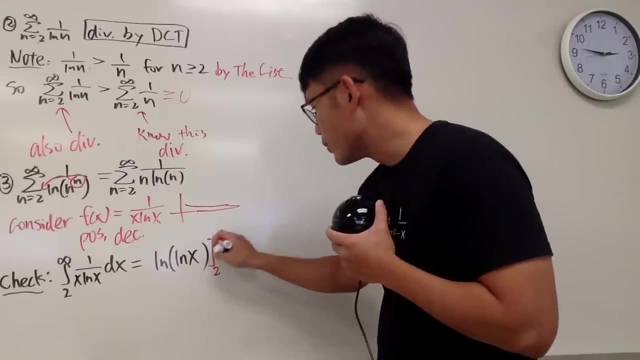 So that's pretty much it. and differentiate that. you get that. so that's pretty much it. We can do. u sub up to, u just write down all the work, Alright. so we have this and we go from 2 to infinity and 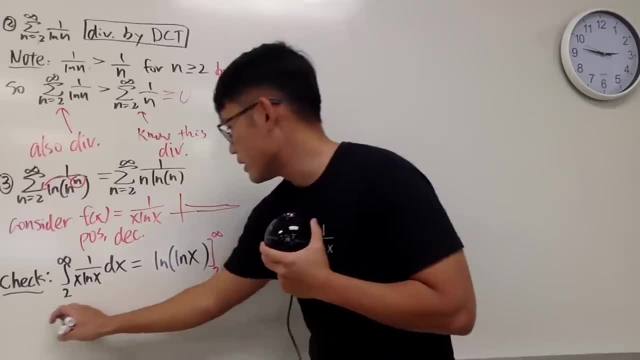 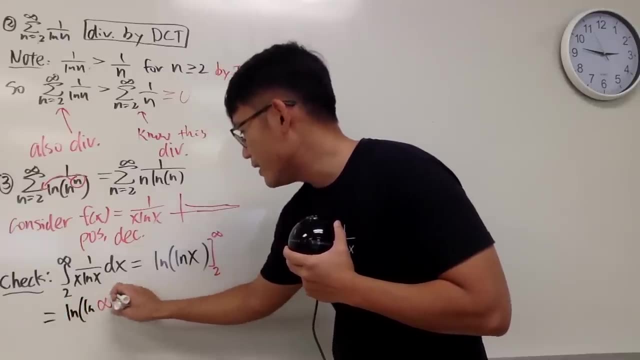 we will see that this right here. let me just put this down so I have more space for that part. Putting infinity, namely we get ln of ln of infinity and then we have to subtract Putting 2: right here we have ln. 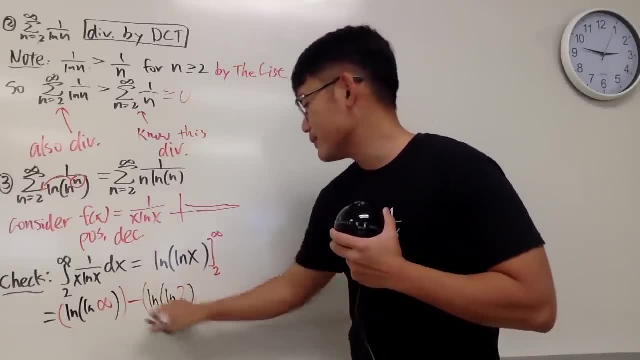 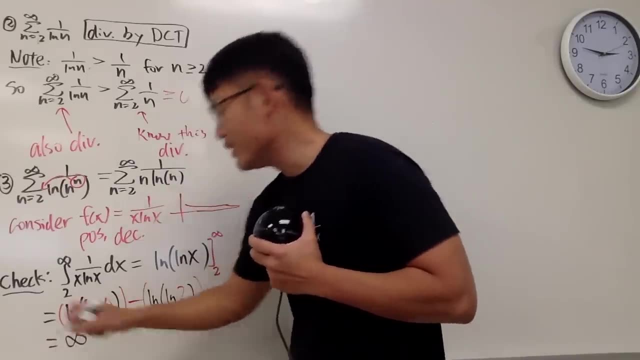 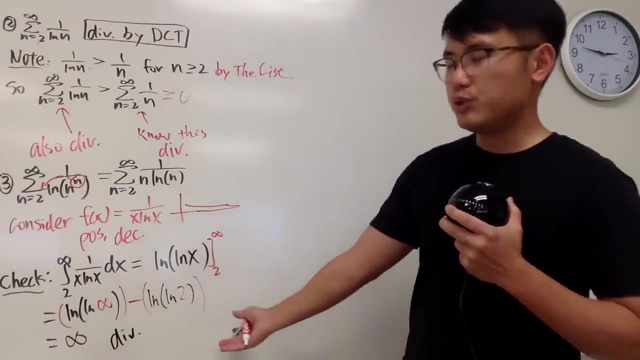 of ln of 2. Like this? Well, well, this right here is finite, this is infinity. infinity minus finite we get infinity. So in another word, this improper integral diverges. And whenever we have this situation, we can go back to the series version. 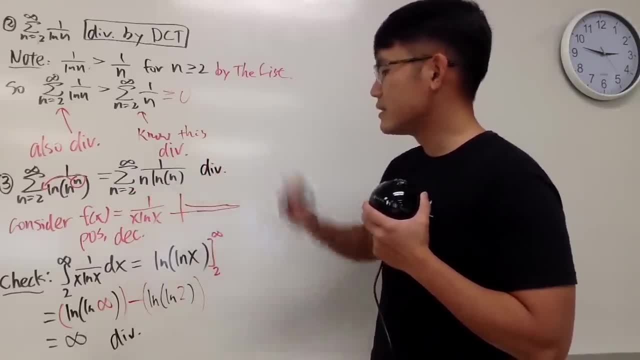 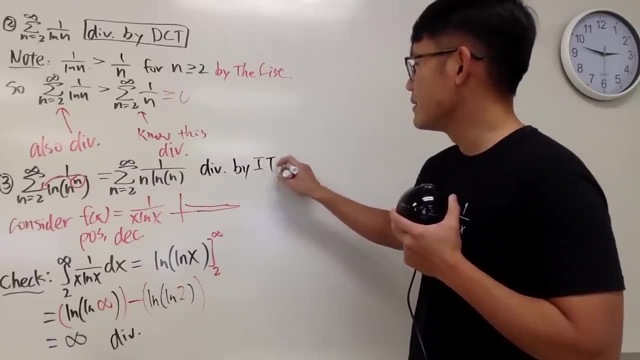 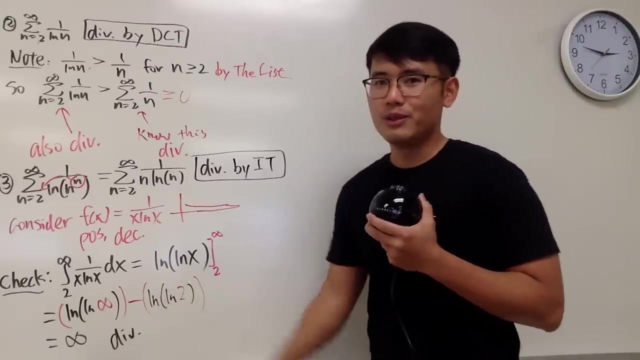 right here and say this right here also diverges Why? By the integral test. So I just put an it for this, an it By it. I think you should spell it out by: like I'm doing 100 of this, so excuse me. 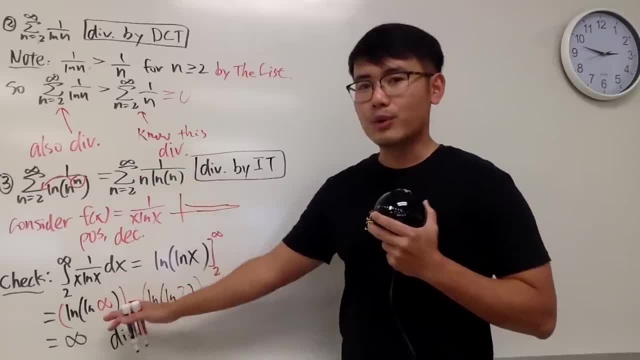 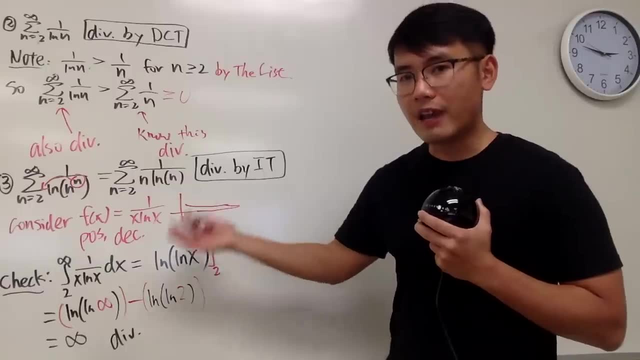 And the truth is, you can draw the same conclusion in terms of their convergency. alright, The idea is that either they will both converge or they will both diverge, But if they converge, they may not converge to the same value, so just keep that in mind. 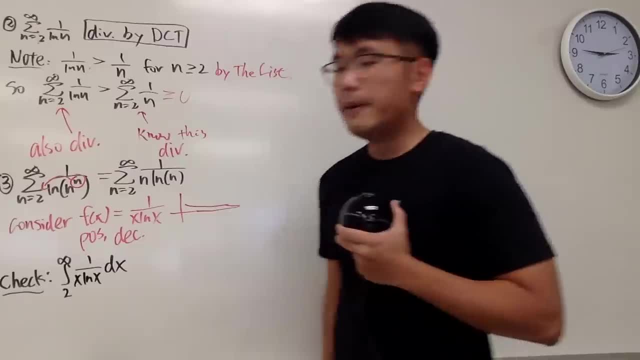 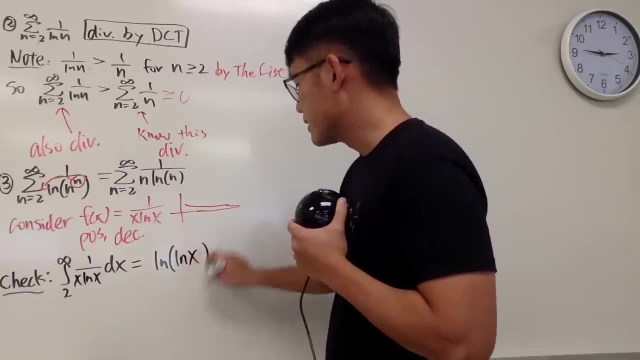 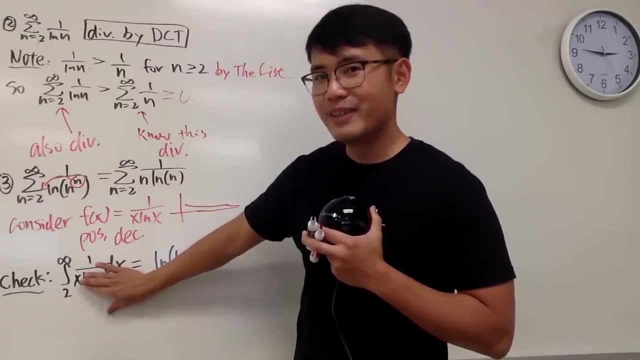 1 over x, ln, x, dx. Well, I will just tell you guys that when you integrate that, we get ln of ln x. Why? Because if you let u equal to ln x, the derivative of ln x is 1 over x, right. 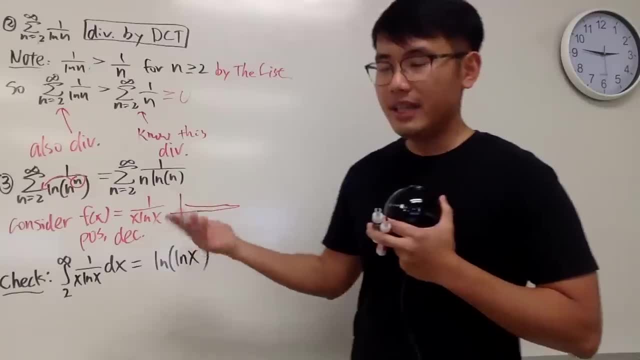 So if you just get it so that you end up with 1 over u and the integral of 1 over u is natural log of u, So that's pretty much it. And if you differentiate that, you get that, So that's pretty much. 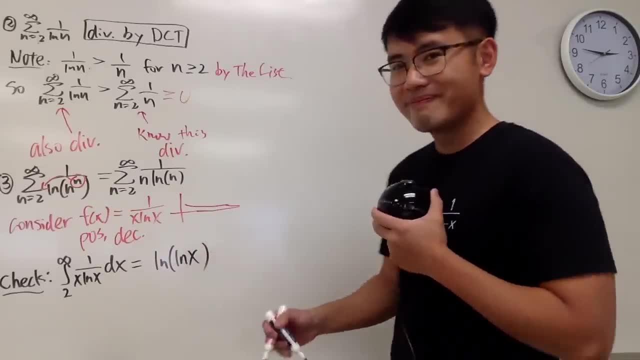 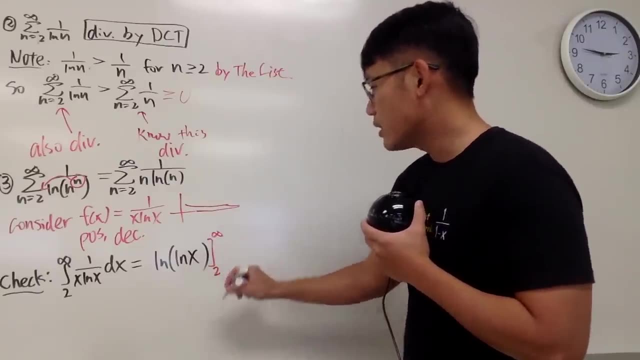 the derivative. Or you can do u sub up to, u Just write down all the work, Alright. so we have this and we go from 2 to infinity and we will see that this right here. let me just put this down. so I have 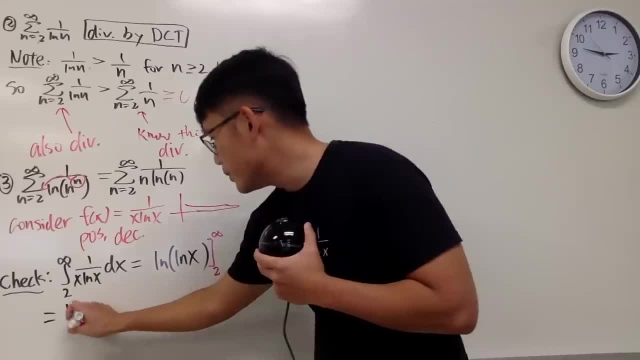 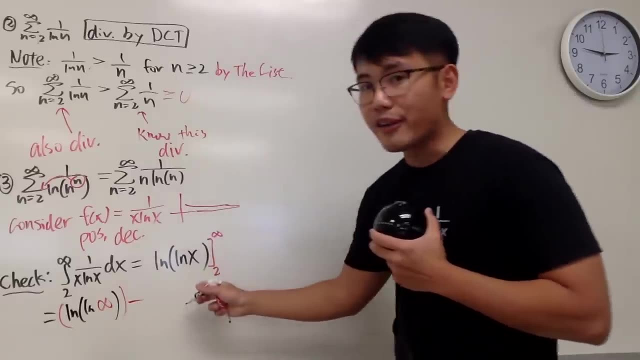 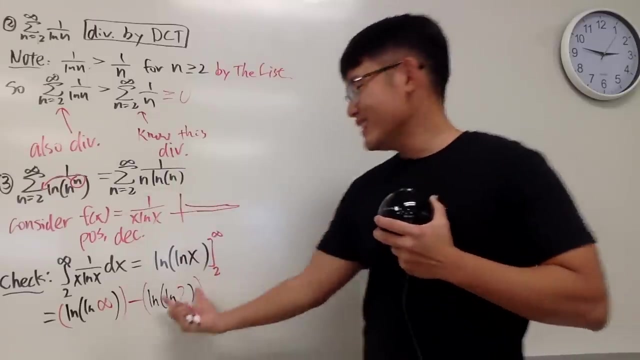 more space for that part. Putting infinity, namely we get ln of ln of infinity, and then we have to subtract, Putting 2, right here, we have ln of ln of 2.. Like this, Well, well, this right here is finite, This is infinity, Infinity minus. 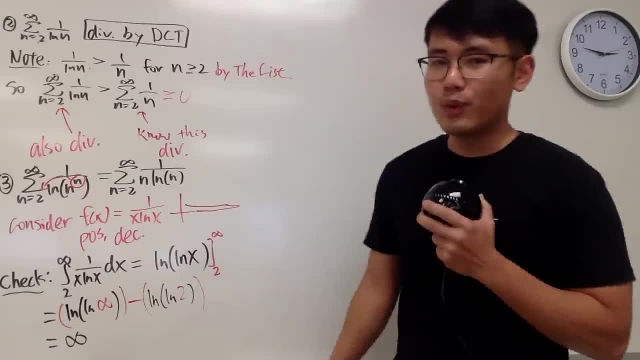 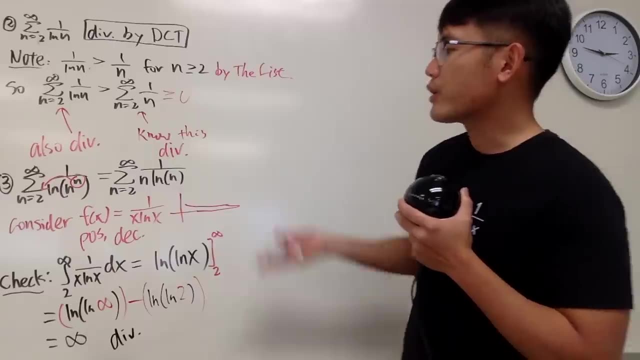 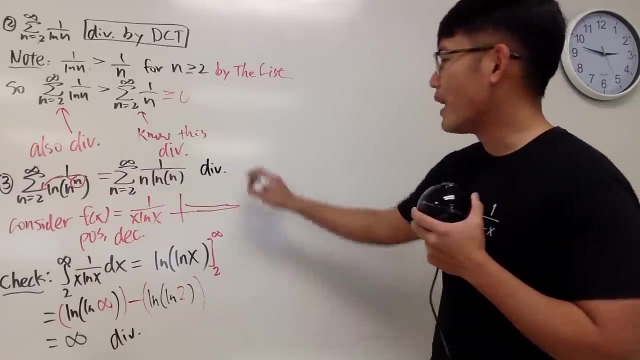 finite, we get infinity. So, in other words, this improper integral diverges And whenever we have this situation we can go back to the series version right here and say this right here: also diverges Why By the integral test. 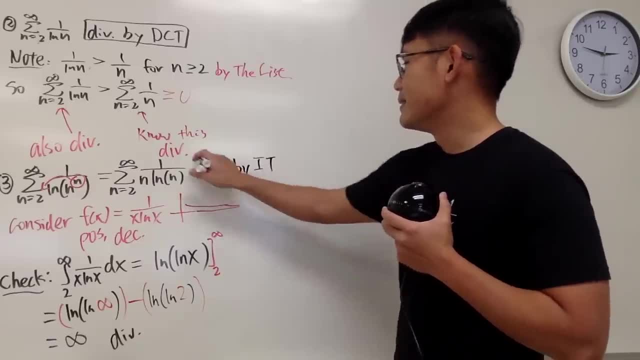 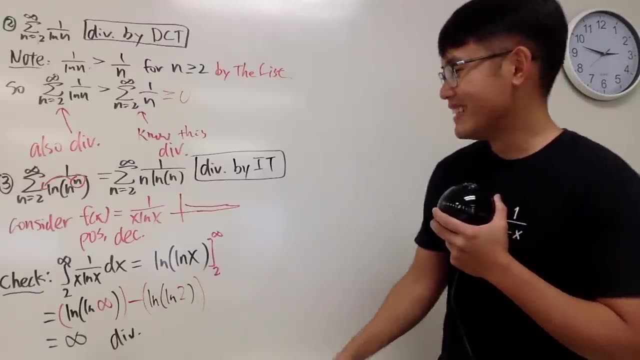 So I just put an i t for this i t By it. I think you should spell it out, but like I'm doing 100 of this, so excuse me. And the truth is, you can draw the same conclusion in terms. 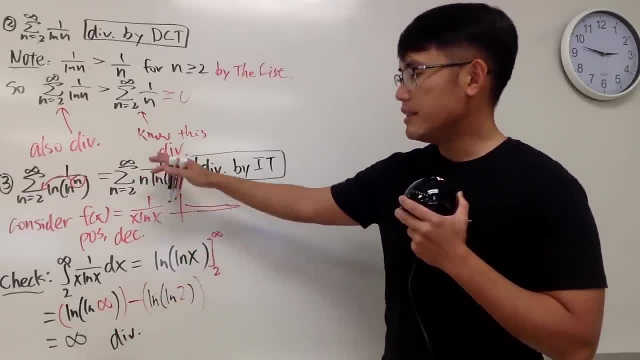 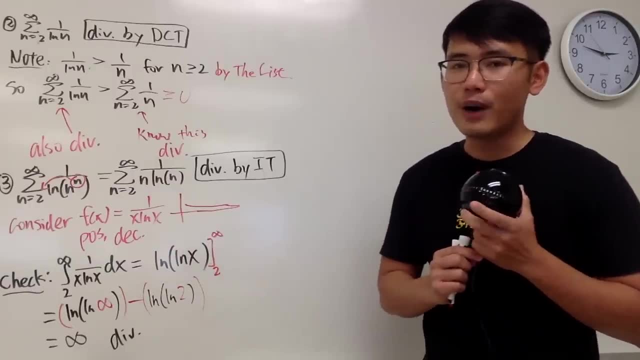 of their convergency. alright, The idea is that either they will both converge or they will both diverge. But if they converge, they may not converge to the same value. so just keep that in mind, Anyway. so that's it for number. 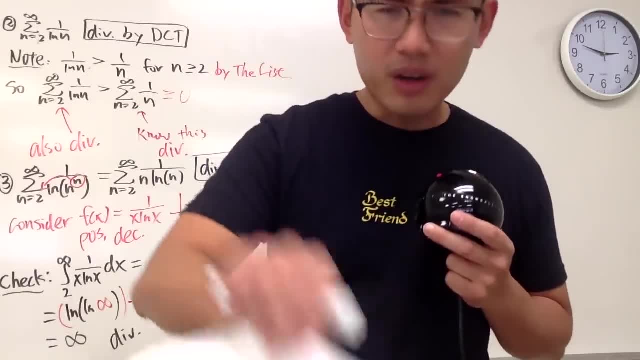 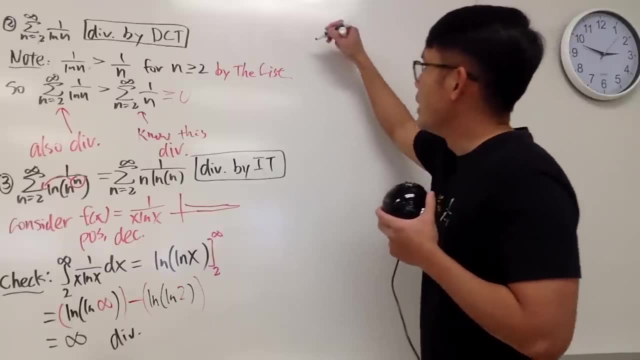 3.. Now moving on to number 4.. Oh my god. Natural log of n, to the natural log of n's power. Anyway, we can do it, No big deal. Here we go. The sum as n goes from 2 to infinity. 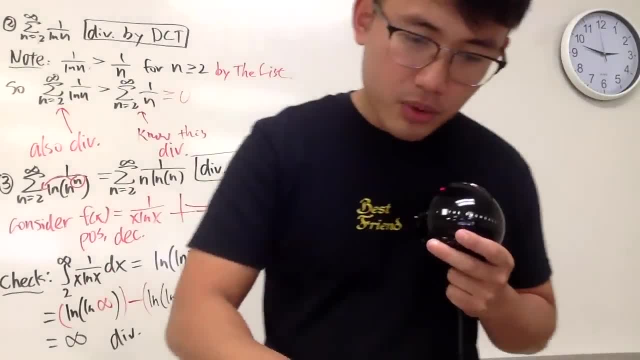 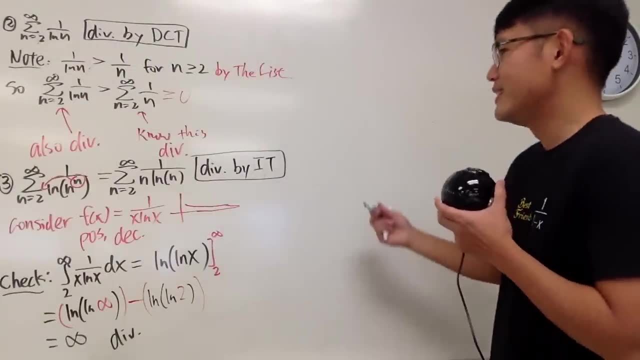 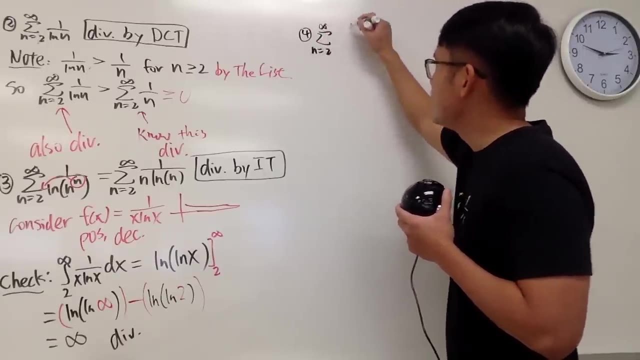 Anyway. so that's it for number 3.. Now moving on to number 4.. Oh my god, ln to ln is power. Anyway, we can do it No big deal. Here we go. The sum as n goes from 2 to infinity. 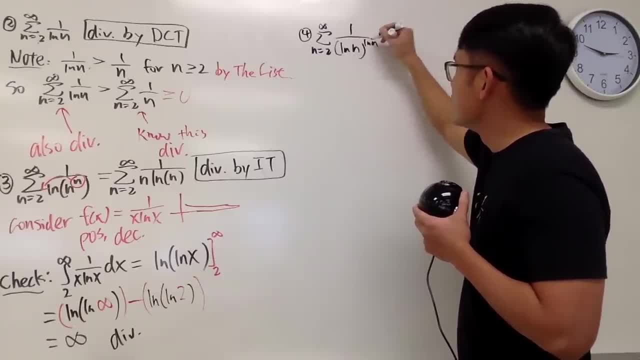 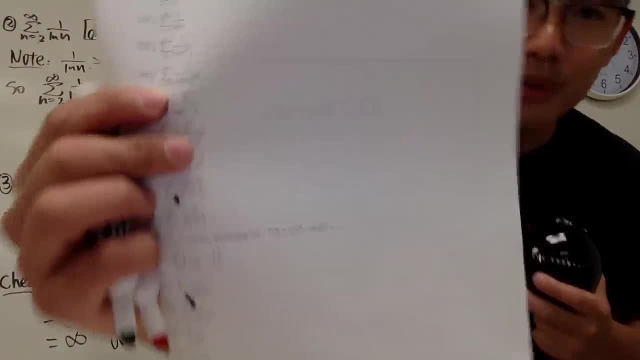 1 over natural log of n raised to the natural log of n, like this, And in fact this is not going from 2 to infinity. If you look at this carefully, I put down 16, 19.. So I would actually like to change this. 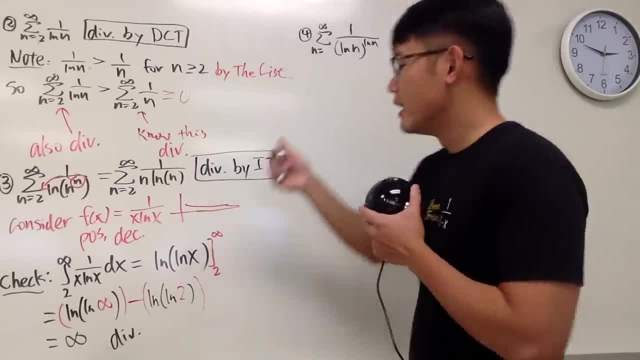 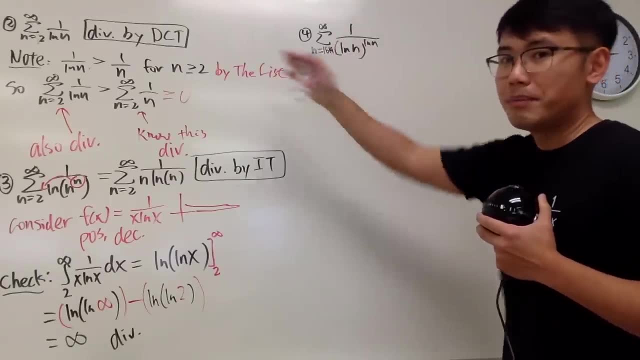 a little bit, You guys will see why. Again, the starting shouldn't bother you too much, but as long as it's not bad. like, for example, n is equal to 1, it would be bad for this situation. As long as it's not bad starting. 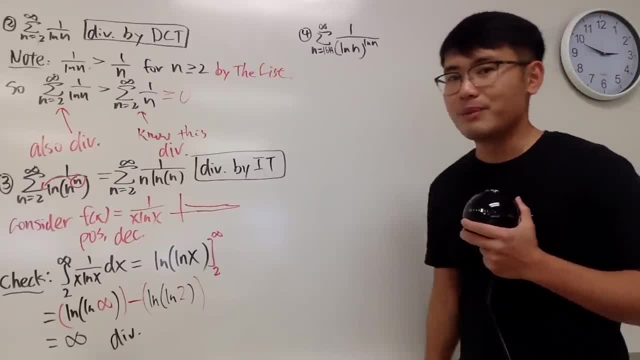 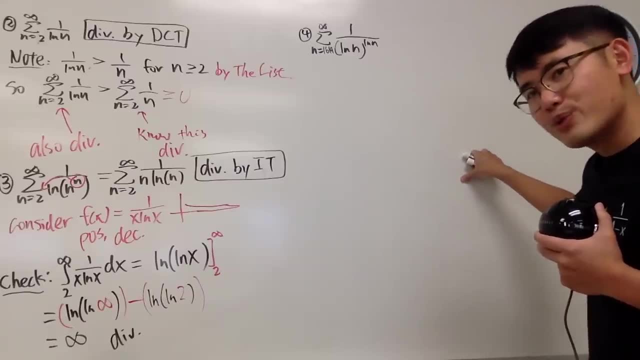 value. in terms of convergence, it doesn't really matter, right? So I can put down like 2019 if I want as well. Oh my god, What should we do? Ah, so many ln questions, Hmm. 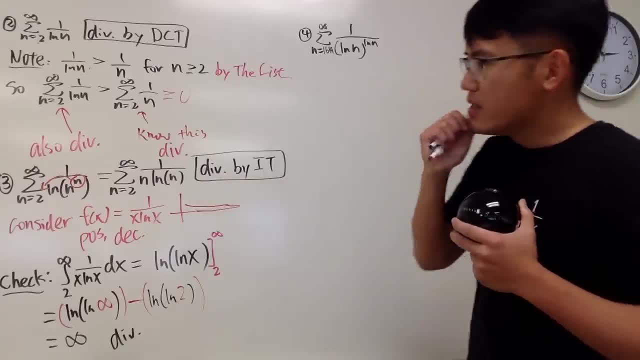 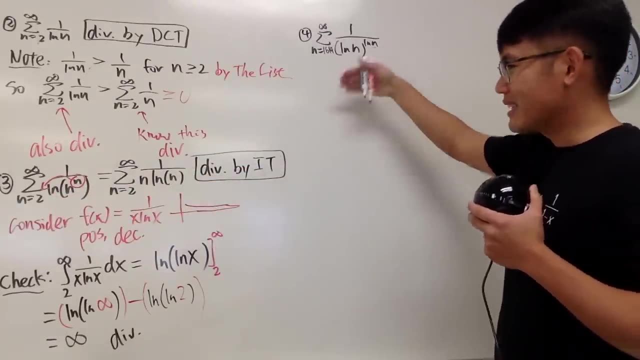 Does this have anything to do with that? You see, earlier we put the biggest in the ln into the smallest and now it's like we put the ln the smallest into, like the biggest ln into the ln power. By the way. 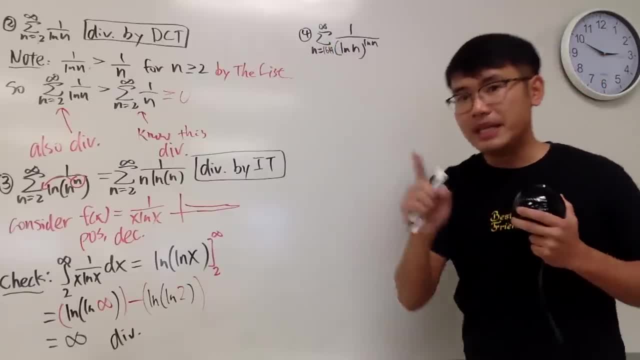 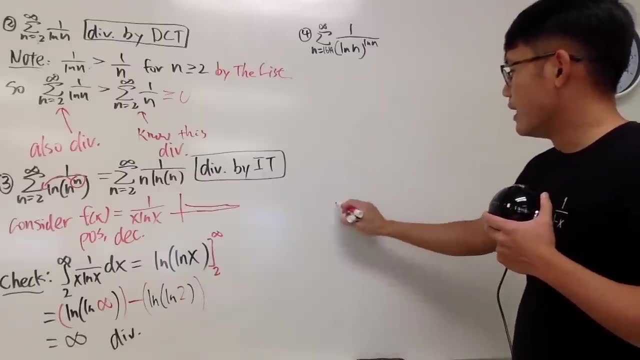 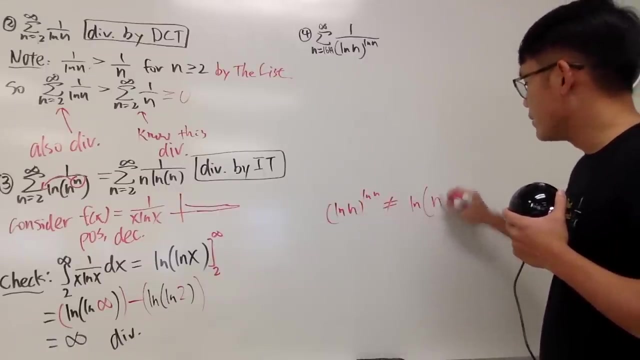 in this case we cannot put the ln in the front because this ln- I should have put down too many parentheses- This right here: ln n to the ln n. this is not the same as saying ln of n to the ln power right This. 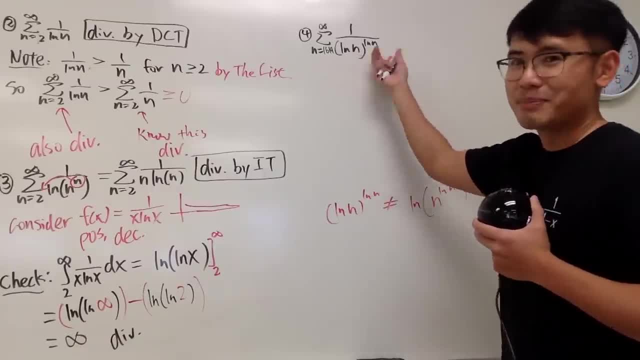 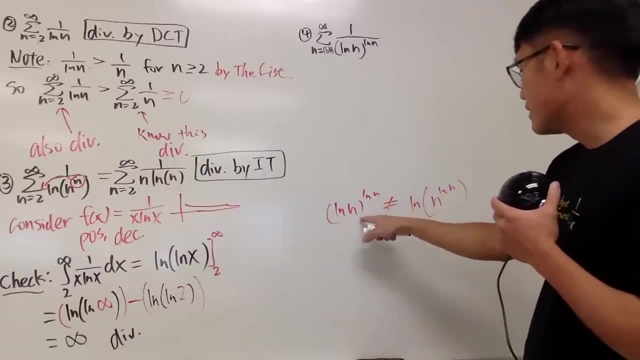 are not the same, So just power function. I wanted to say you keep this space and multiply by itself ln time, but that doesn't make sense. So excuse me on that, But just know that this is not the same. 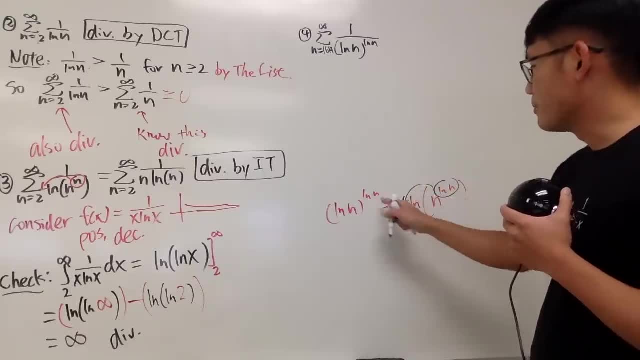 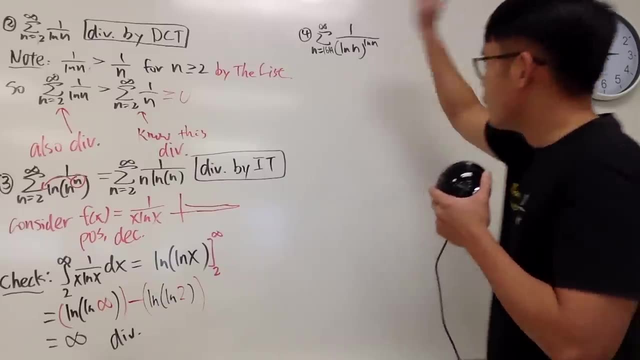 Right, So you cannot. This right here is okay, to bring that to the front, but this right here you cannot. So keep that in mind, Well, well, Now here is the. DO We have the base being ln n? We don't. 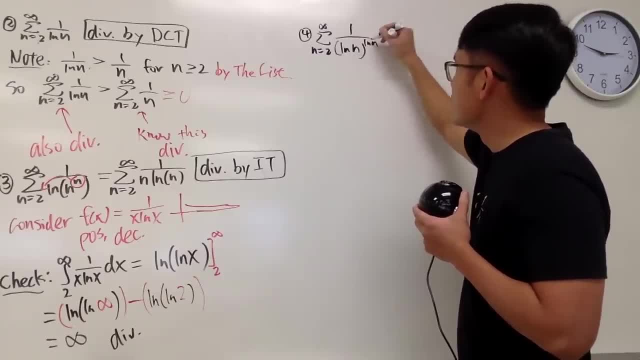 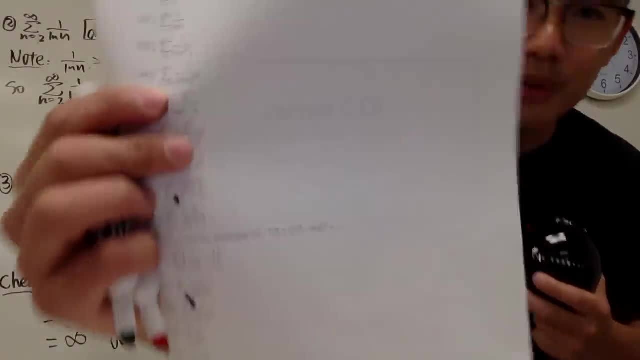 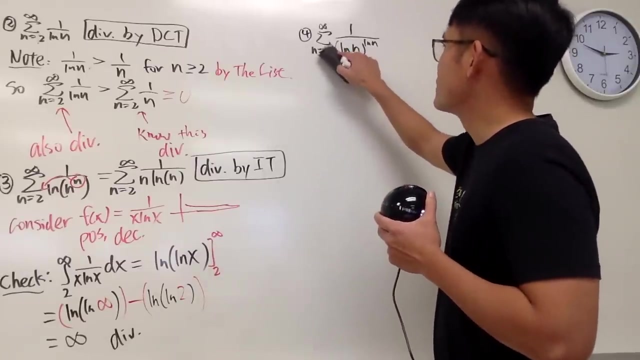 1 over ln raised to the ln like this, And in fact this is not going from 2 to infinity. If you look at this carefully, I put down 16, 19.. So I would actually like to change this a little bit. You guys will see why. 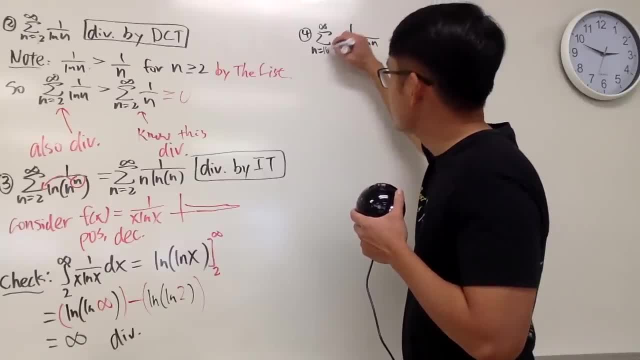 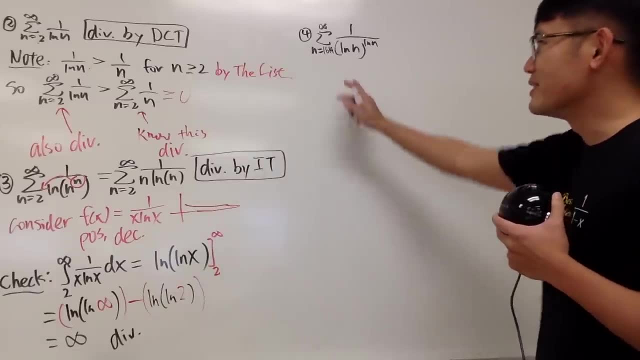 Again, the starting shouldn't bother you too much, but as long as it's not bad. like, for example, n is equal to 1, it would be bad for this situation, As long as it's not a bad starting value. 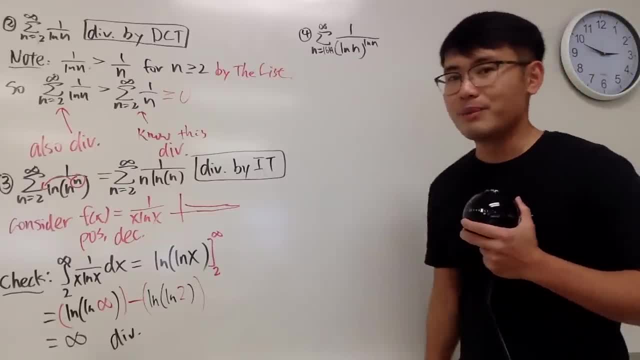 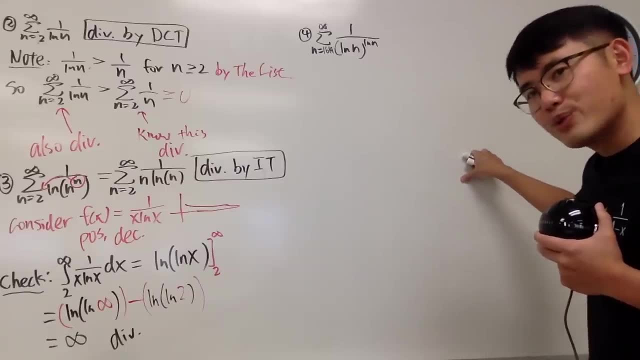 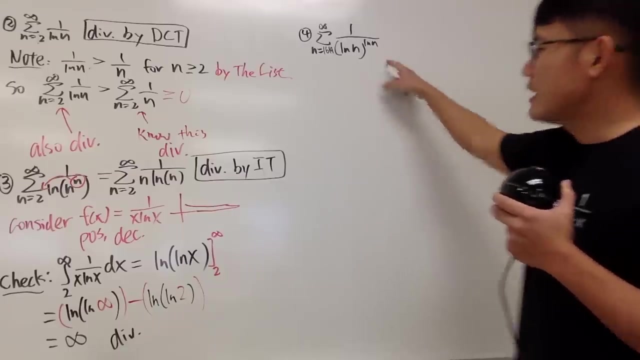 in terms of convergence, it doesn't really matter, right? So I can put down like 2019 if I want as well. Oh my god, What should we do? Ah, so many ln questions. Hmm, Does this have anything? 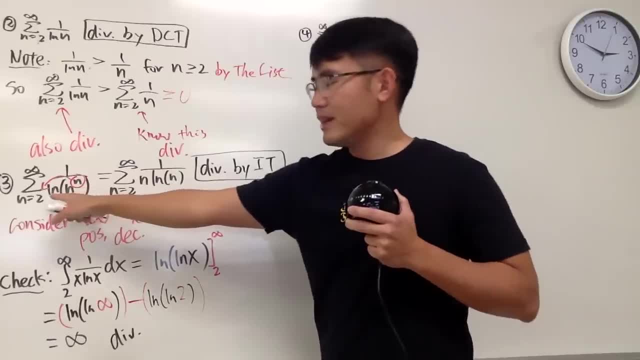 to do with that. You see, earlier we put the biggest in the ln into the smallest and now it's like we put the ln the smallest into like the biggest, like ln n to the ln power. 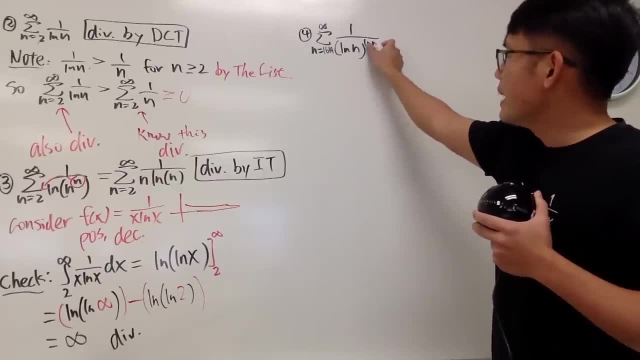 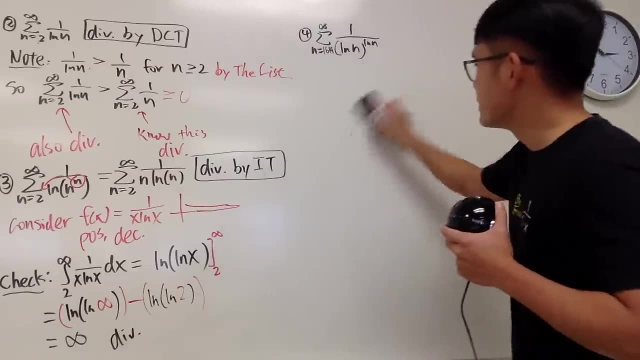 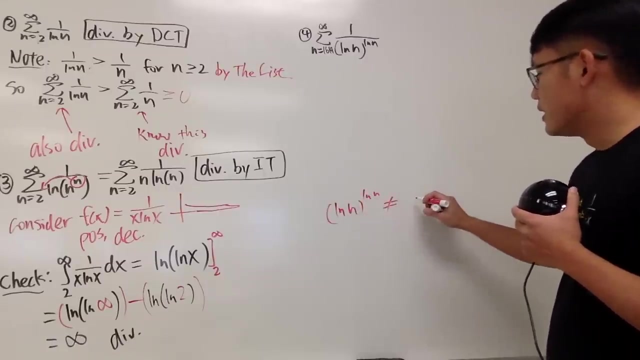 By the way, in this case we cannot put the ln in the front, because this ln. I should have put down too many parentheses. This right here: ln? n to the ln n. this is not the same as saying ln of n to the ln. 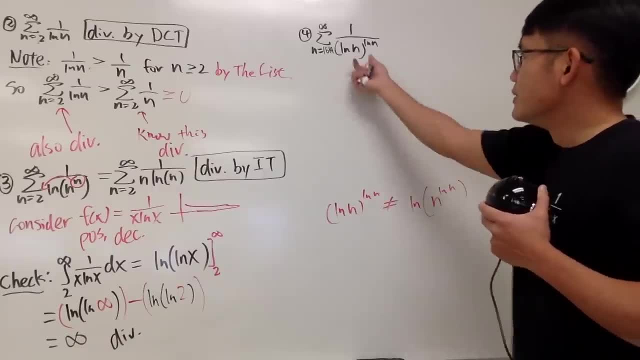 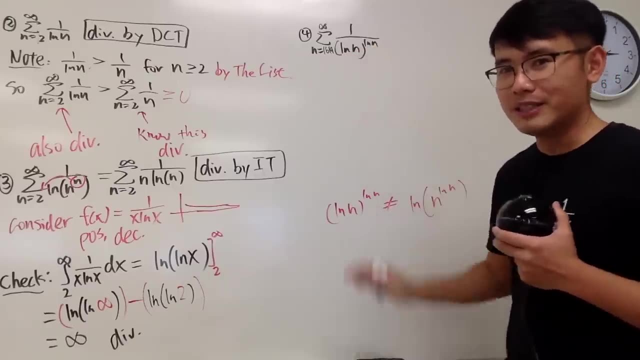 power. right, This is not the same. So just power function. I wanted to say you keep this base and multiply by itself ln time, but that doesn't make sense. so excuse me on that. But just to note that this is not the same. 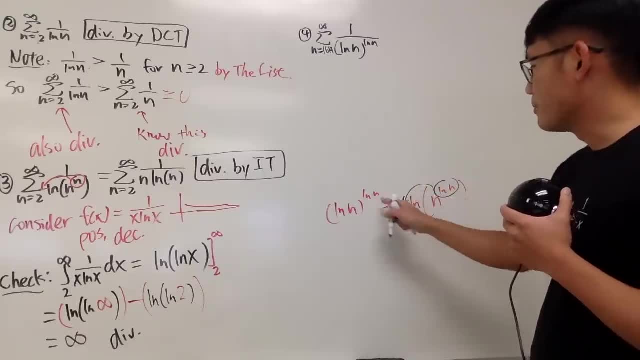 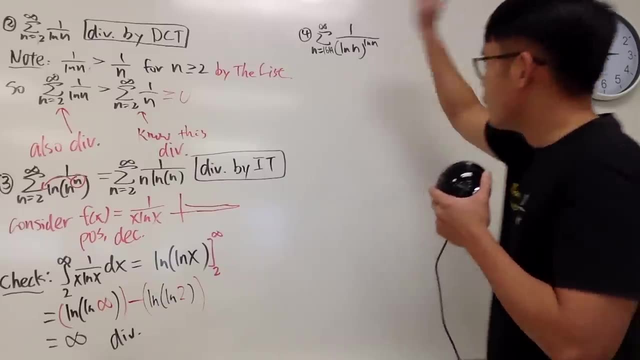 So you cannot. this right here is okay, to bring that to the front, but this right here you cannot. so keep that in mind, Well. well, Now here is the. DO We have the base being ln n? We don't. 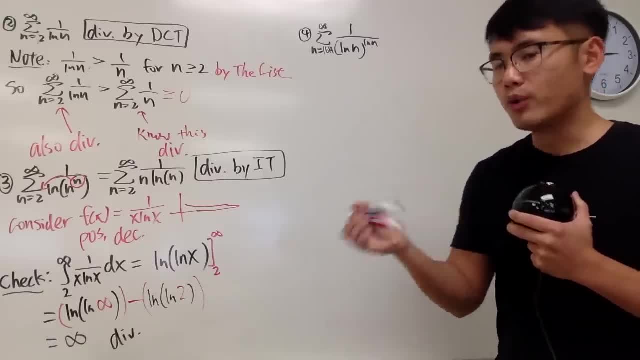 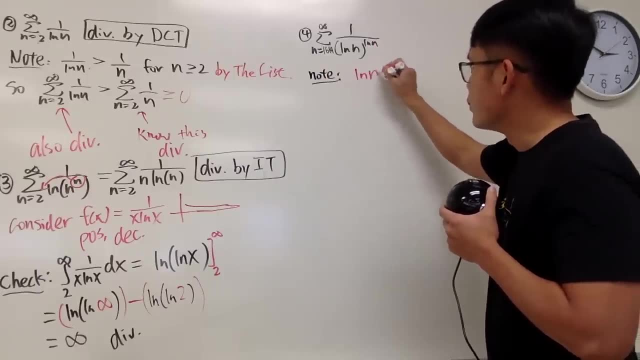 like that. We usually like to work with space e, so here we go. Let me just put down a note right here for you guys. Let's look at this ln n in red and then raise to the ln n's power. Well, can I write? 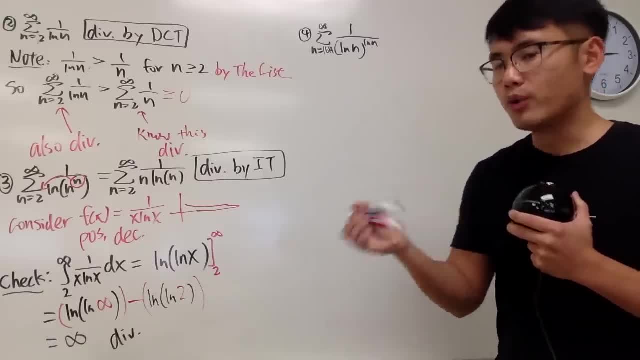 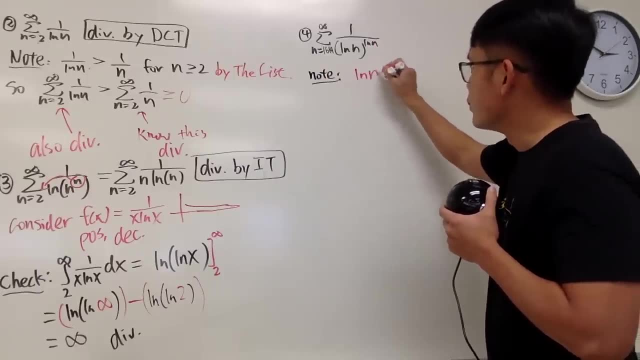 like that. We usually like to work with space e, So here we go. Let me just put down a note right here for you guys. Let's look at this ln in red and then raise to the ln n's power. Well, can I write? 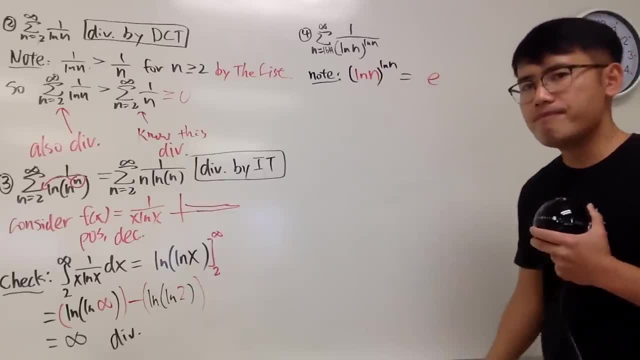 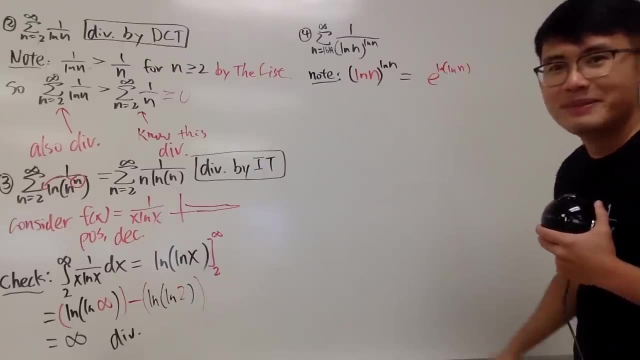 the base as e to the power. Hmm, I think so I just have to put ln of whatever. this is again Right, Because you see this e and this ln on the outside they cancel. We just have ln n back. 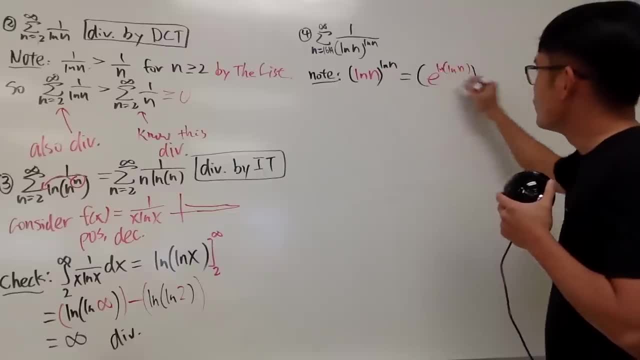 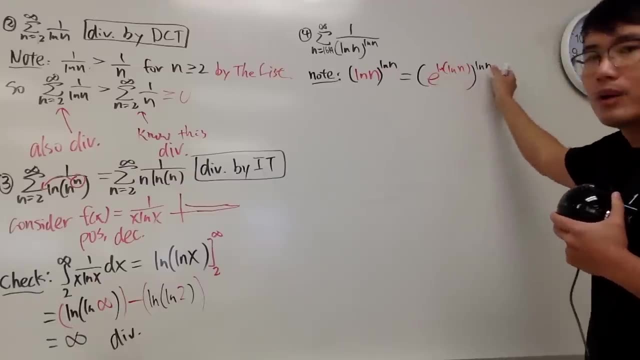 So that's still inside. So we have this, and then we take this again, raise to the ln n's power And now check this out. We have this to this power, to that power. we can multiply the powers together. So if you would like, I will write down one more. 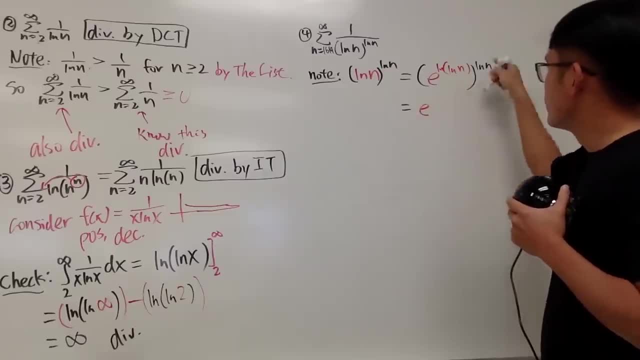 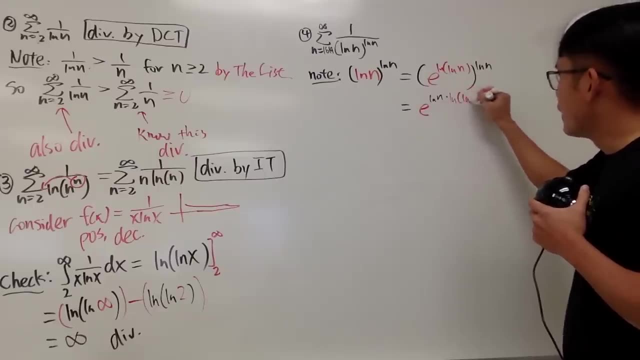 step right here. I can write down this as: e to the ln n's power, and of course, this power is multiplying with that power: ln of ln n like this. Well, this time, what we will do is we will pair this up. 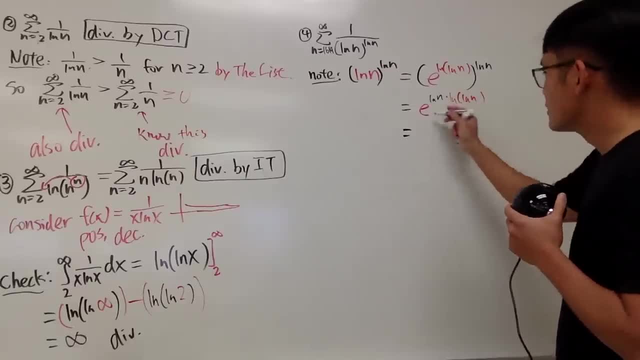 as the base, and then that will be the power. So we actually end the hub. Let me just put this down in black, So I'll change the e to black as well, like this e to the ln n inside, and then we will raise this. 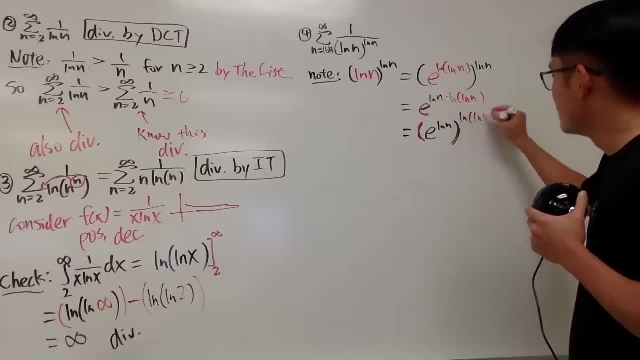 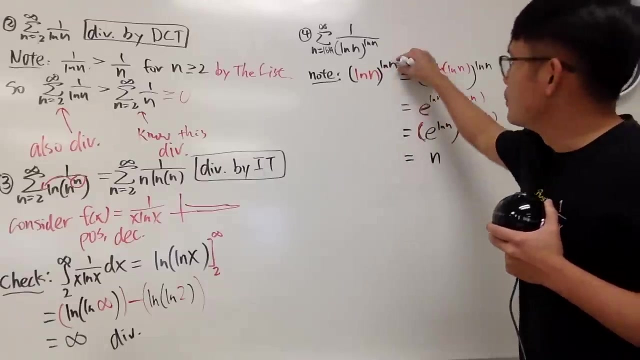 We'll raise this to the ln ln n power like that. Okay, And the beauty of that is e to the ln n is n. I know The idea is that, in fact, this is a log property. You can put whatever. 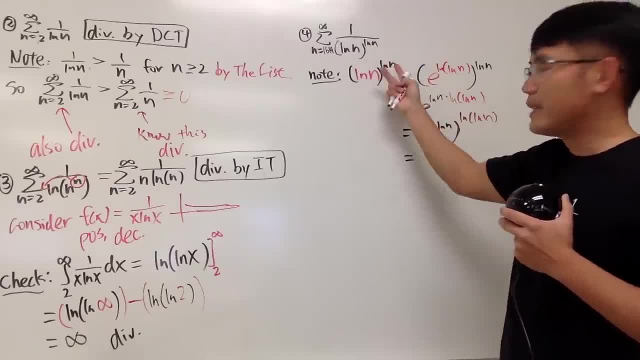 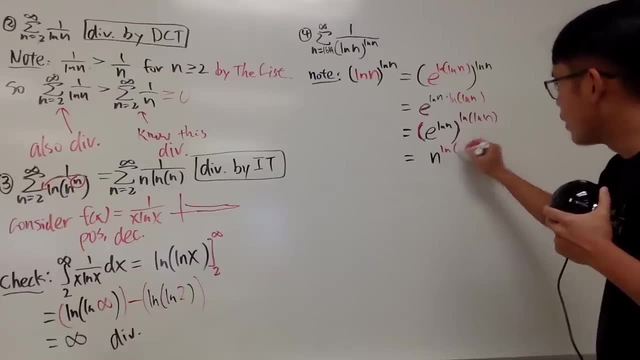 inside, here, in here, and then just switch this and that like that. That's exactly a proof right here. Anyway, this right here is just n, and of course, you still keep the ln of ln n power like this. So cool, isn't it. 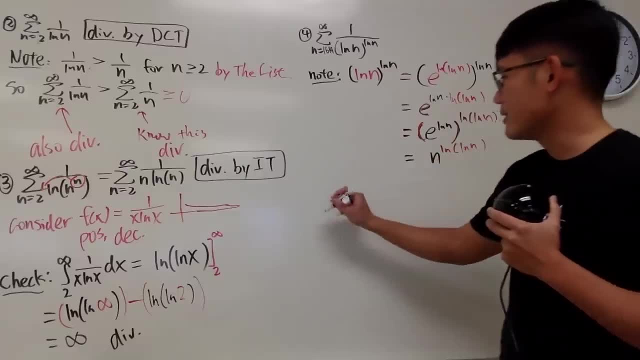 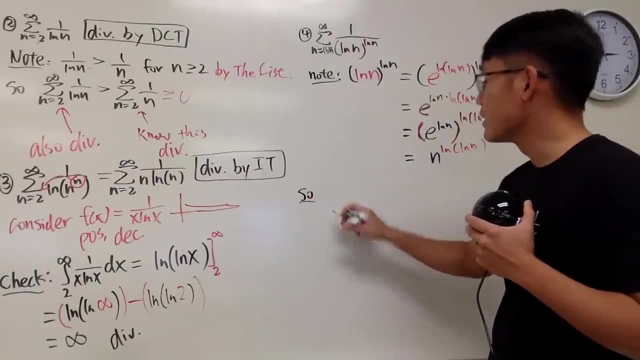 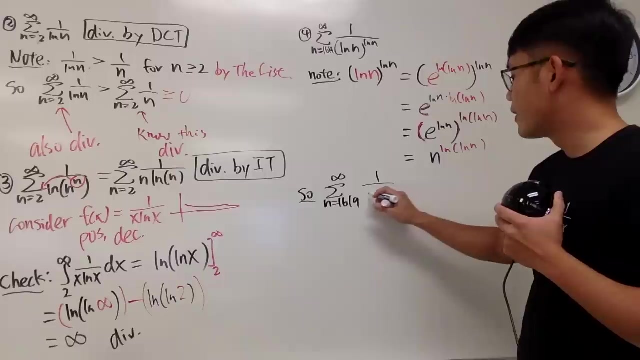 Now here is the deal. I will just continue to write down this right here. So note: the base. is that right? So we have the following: The sum as n goes from 16, 19 to the infinity's power, 1 over. 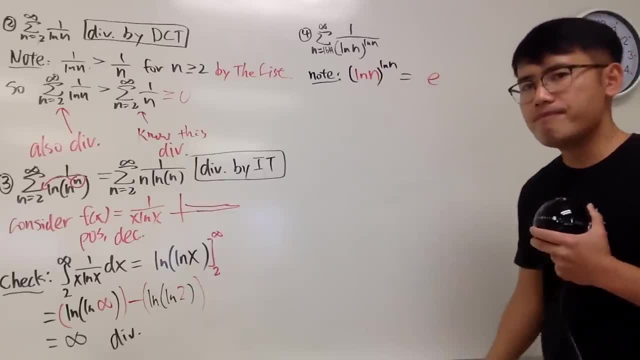 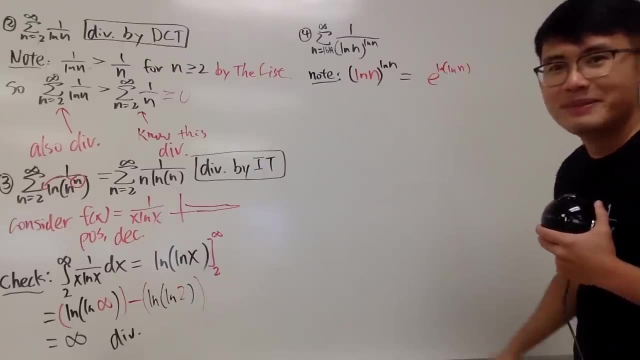 the base as e to the power. Hmm, I think so I just have to put ln of whatever. this is again Right, Because you see this e and this ln on the outside they cancel. We just have ln n back. 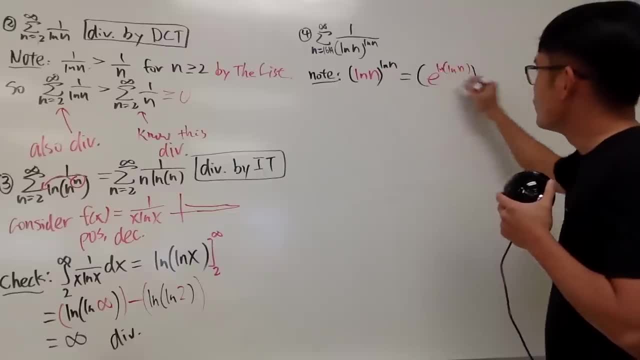 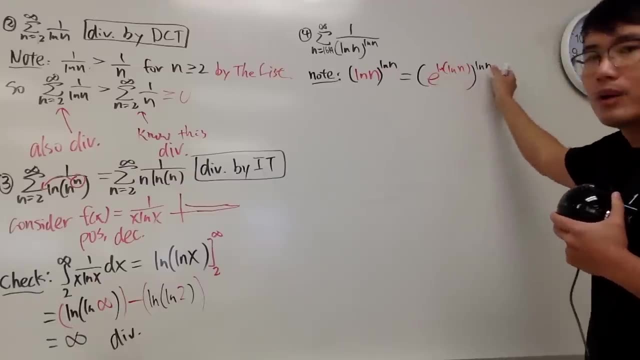 So that's still inside. So we have this, and then we take this again, raise to the ln n's power And now check this out. We have this to this power, to that power. We can multiply the powers together. So if you would like, I will write down. 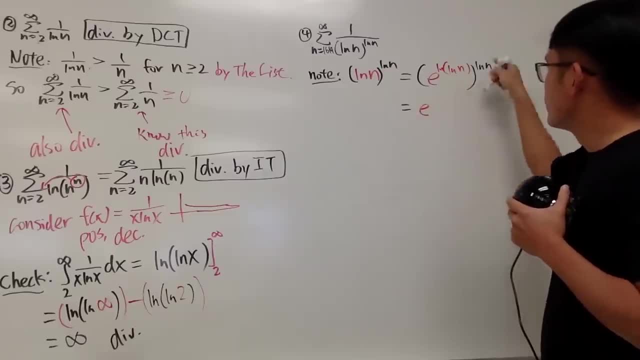 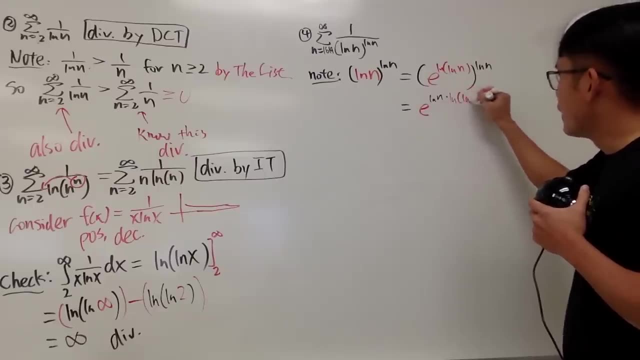 one more step right here. I can write down this as: e to the ln n's power, And of course, this power is multiplying with that power: ln of ln n like this. Well, this time what we will do is we will pair this up. 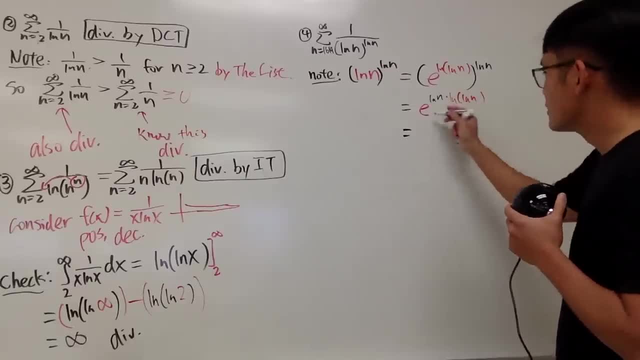 as the base, and then that will be the power. So we actually end up- let me just put this down in black. So we will change the e to black as well, like this e to the ln n inside, and then we will raise this. 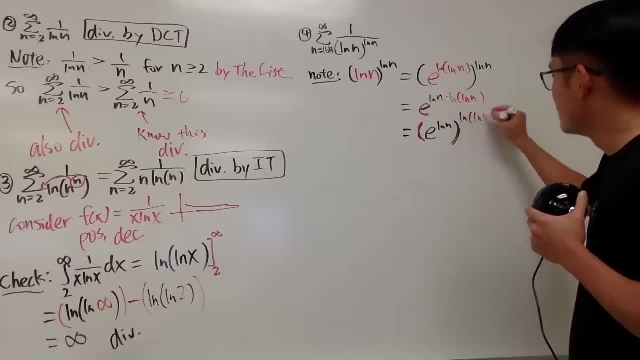 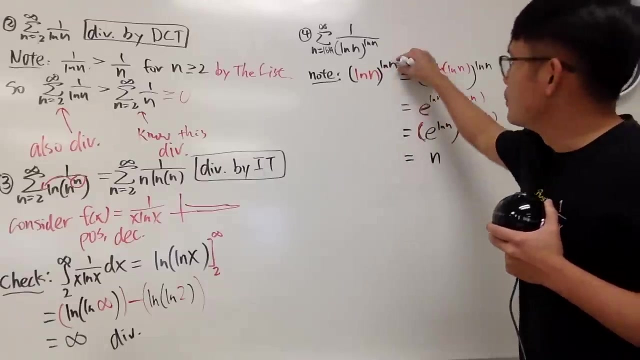 We will raise this to the ln n power, like that. Okay, And the beauty of that is e to the ln n is n. I know The idea is that, in fact, this is a log property. You can put whatever. 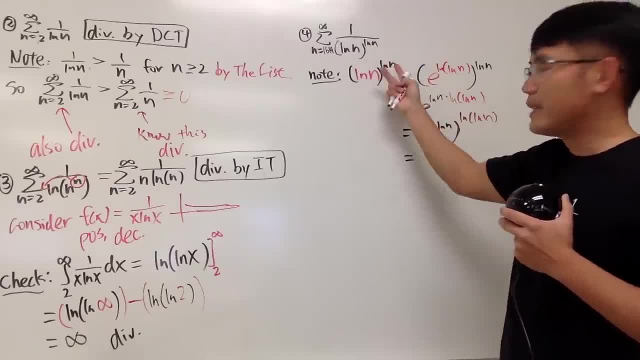 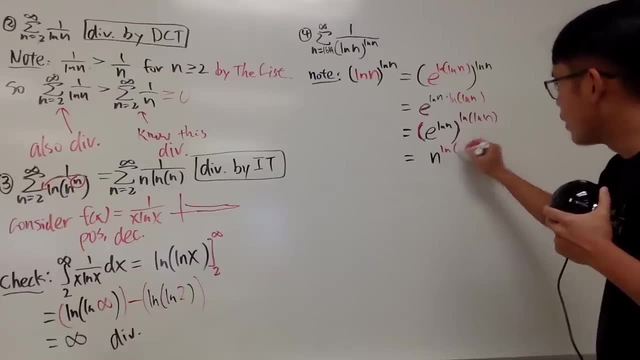 is inside, here, in here, and then just switch this and that like that. That's exactly the proof right here. Anyway, this right here is just n, and of course, you still keep the ln of ln n power like this. So cool, isn't it. 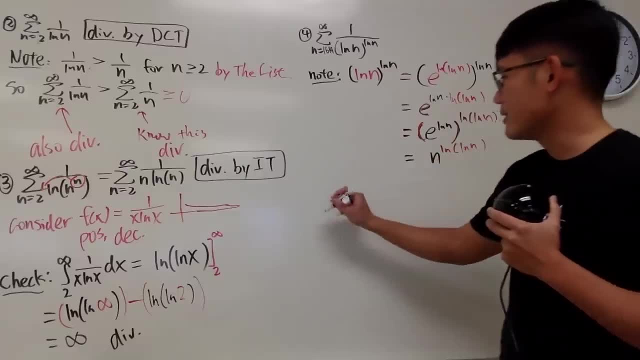 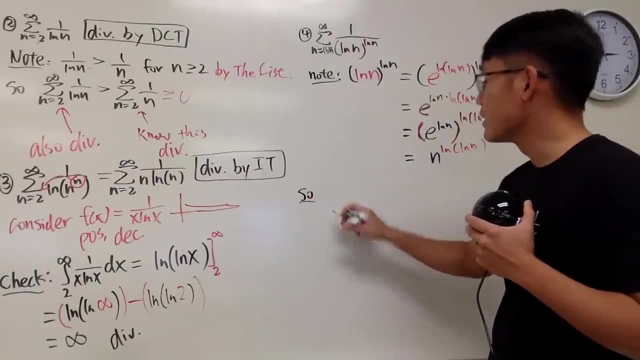 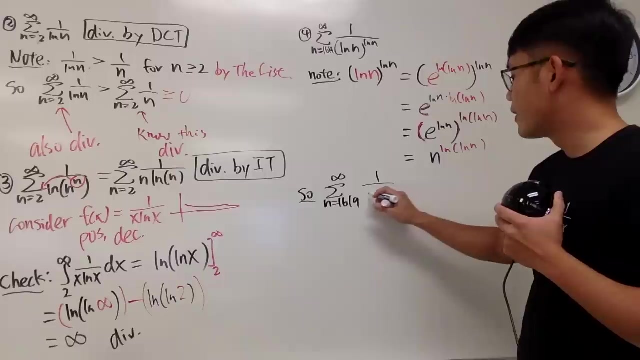 Now here is the deal. I will just continue to write down this right here. So note: the base. is that right? So we have the following: The sum as n goes from 16, 19 to the infinity's power, 1 over ln. 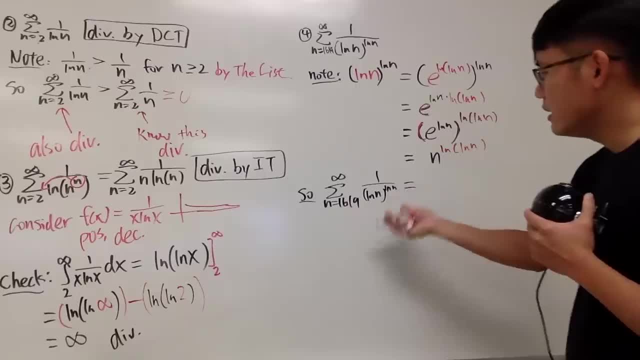 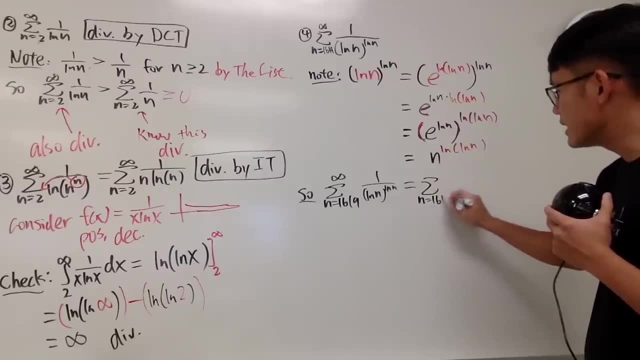 n to the ln n. This, right here, is exactly the same as you replace this for the denominator, which is the sum, as n goes from 16, 19 to the infinity. right here I want to say infinity power, but you know. 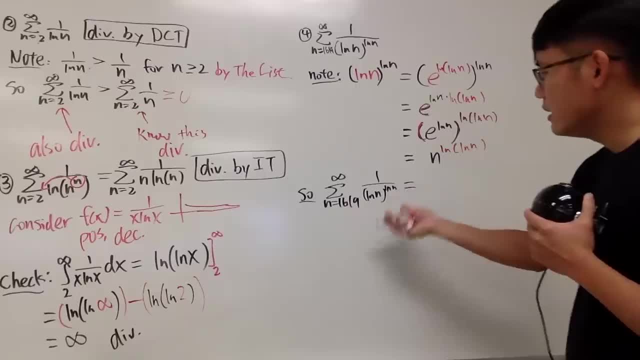 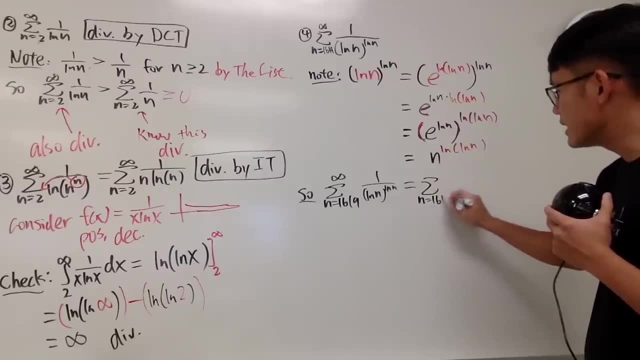 ln n to the ln n. This, right here, is exactly the same as you replace this for the denominator, which is the sum, as n goes from 16, 19 to the infinity. right here I want to say infinity power, but you know. 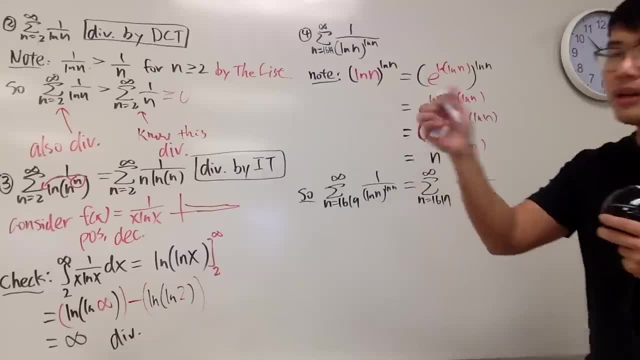 it's not Infinity power. We know there's an infinity stone somewhere on the Earth, but I wish I could find it. If you guys found it, let me know. I'll give you guys like a million dollars Anyway. 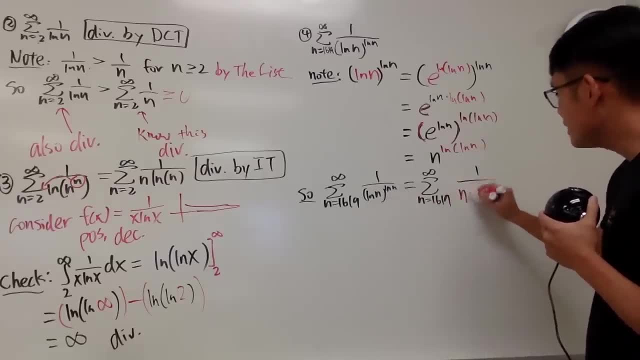 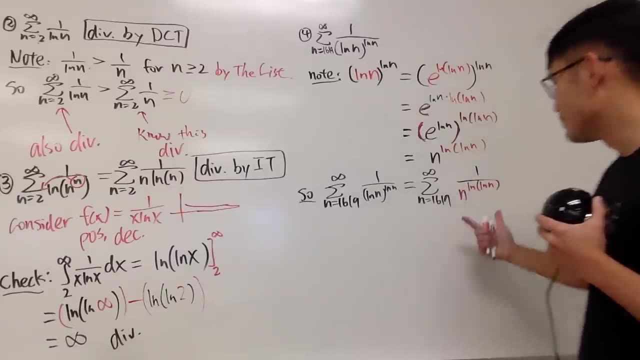 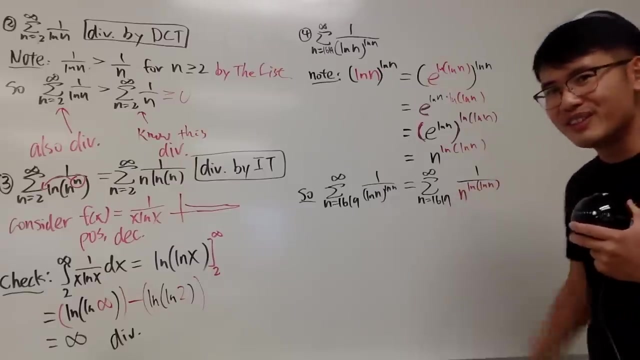 this right here, is that? so I'll just put that down, Namely n to the ln of ln n's power, like that. Now check this out: We have the base right here, being n The power. oh my god, it actually goes to infinity, huh. 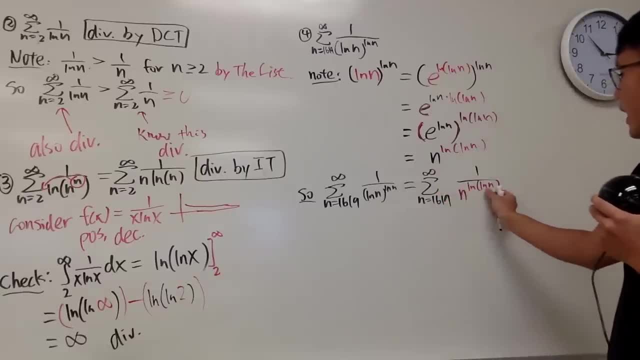 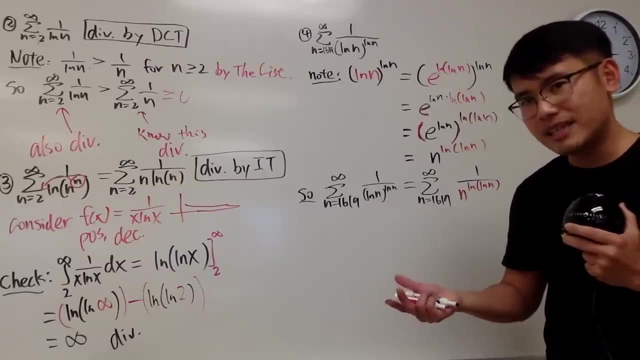 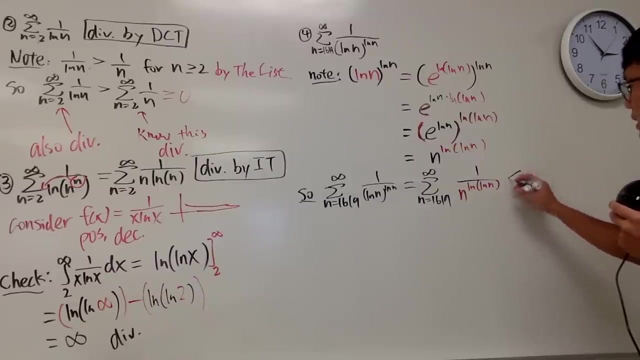 Right, Because if you put n to infinity, ln infinity is infinity, ln infinity is still infinity. That should converge, And to make this slightly more legitimate we will have to say, well, maybe we can do the small check again. I would like to see: 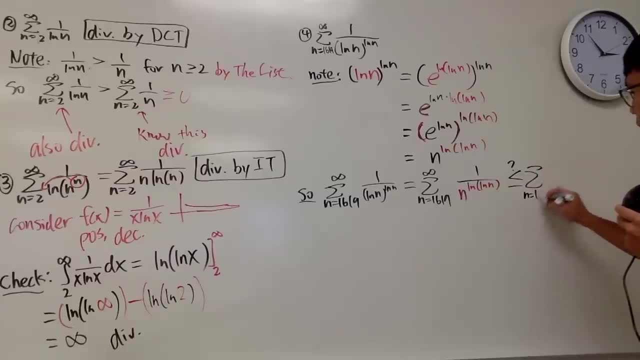 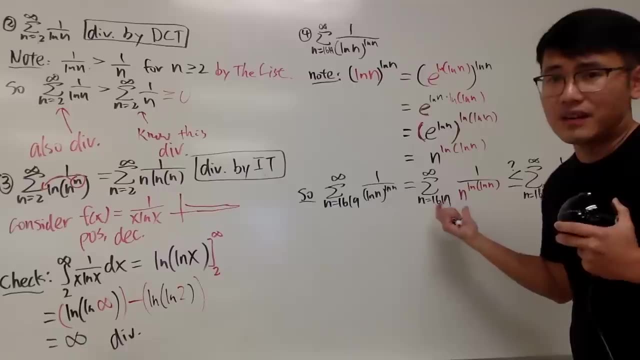 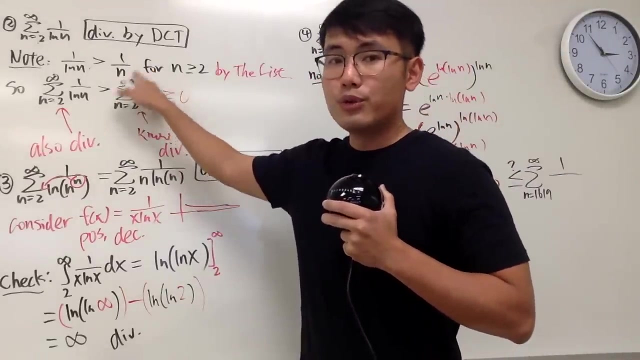 is this less than or equal to the sum, as n goes from 16,, 19 to infinity? right here, And because I think this is convergent, let me use a convergent for it. But we know, hmm, this right here diverges 1 over n to the first power. 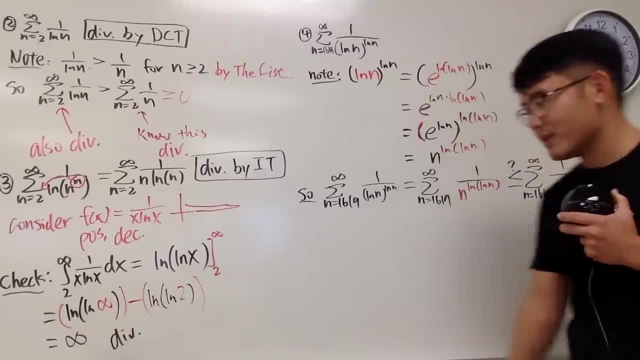 diverges. We don't want to use that. Let's increase the power by another one. So we have ln, We have n squared right here. Let me see if this is true. Well, just do this real quick. Let's do the check. 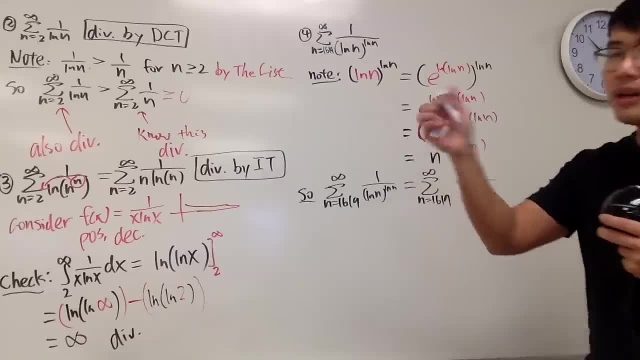 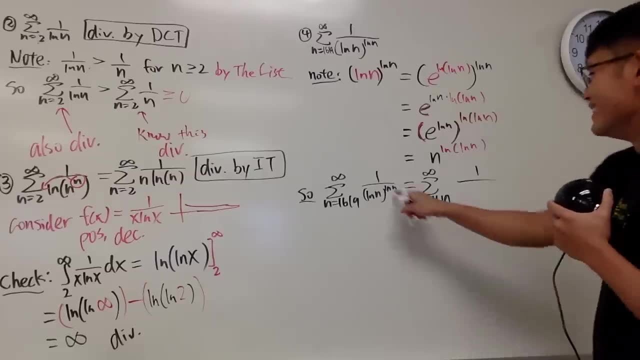 it's not Infinity power. We know there's an infinity stone somewhere on the Earth, but I wish I could find it. If you guys found it, let me know. I'll give you guys like a million dollars. Anyway, this right here is that so I'll. 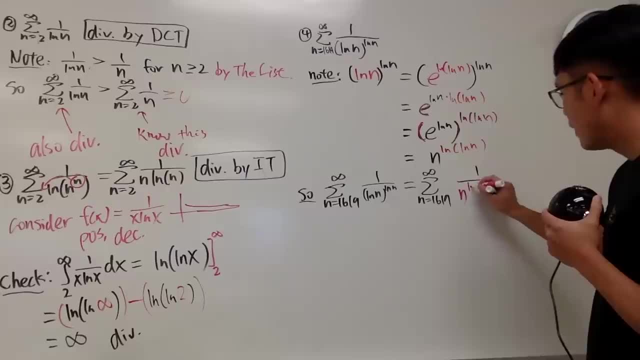 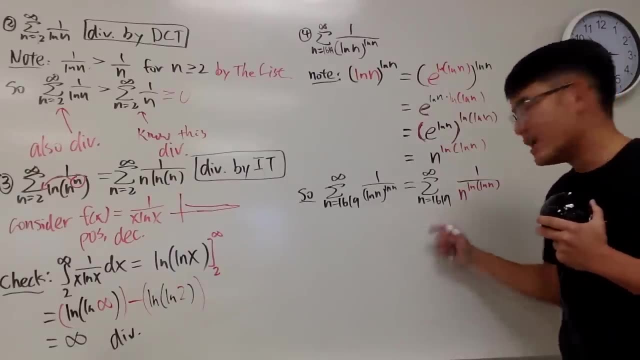 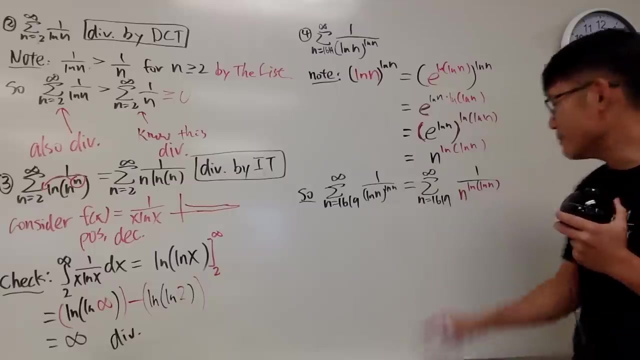 just put that down, namely n to the ln of ln n's power, like that. Now check this out: We have the base right here, being n The power. oh my god, it actually goes to infinity. huh, Right, Because if you, 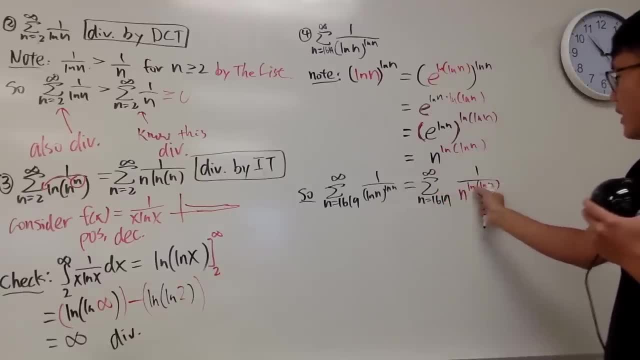 put n to infinity. ln infinity is infinity. ln infinity is still infinity. That should converge, And to make this slightly more legitimate we will have to say: well, maybe we can do the small check again. I would like to see: is this less than or equal to? 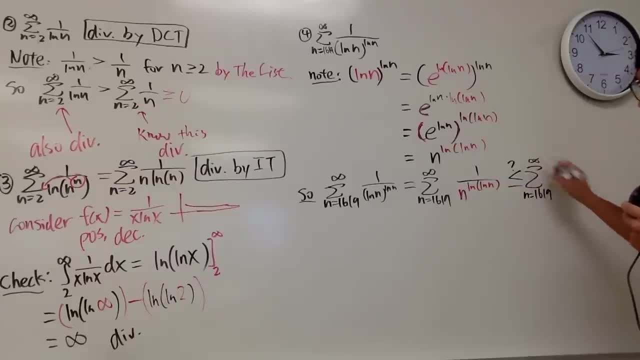 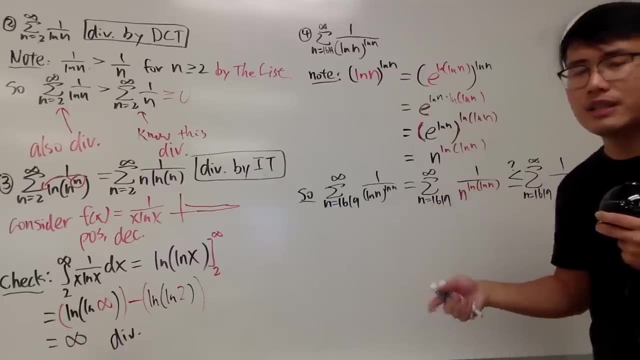 the sum as n goes from 16,, 19 to infinity. right here, And because I think this is convergent, let me use a convergent for it. But we know, hmm, this right here diverges 1 over n to the first power. 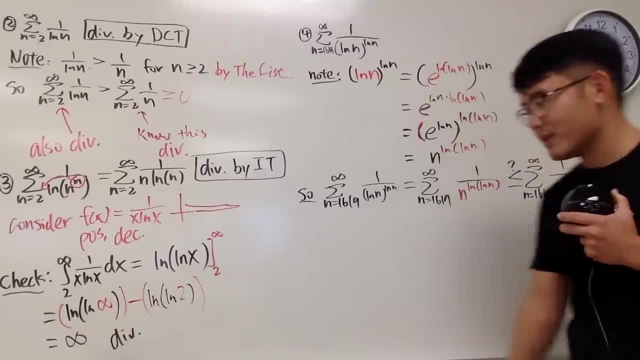 diverges. We don't want to use that. Let's increase the power by another one. So we have ln, We have n squared right here. Let me see if this is true. Well, just do this real quick. Let's do the check. 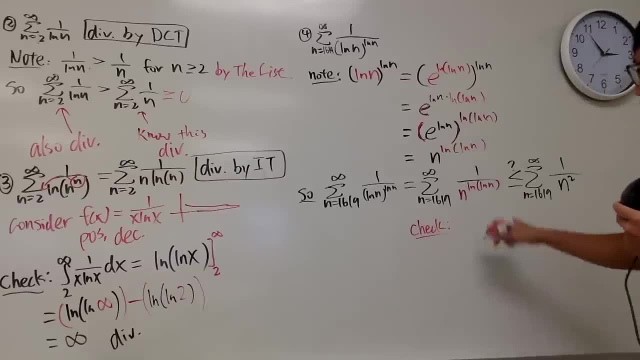 Right here. So, if you would like, you can do the check, which is this. Well, we just have to check 1 over n ln, ln n power. Is this less than or equal to 1 over n squared? You can cross-multiply real quick. 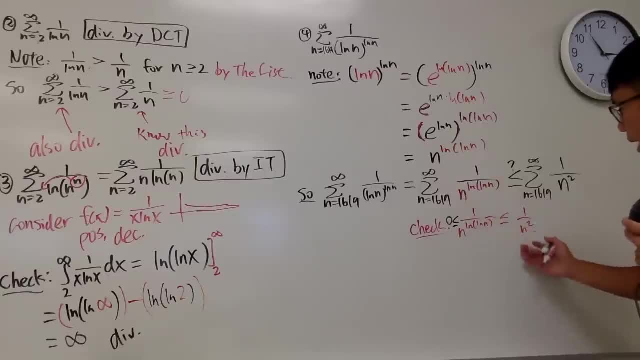 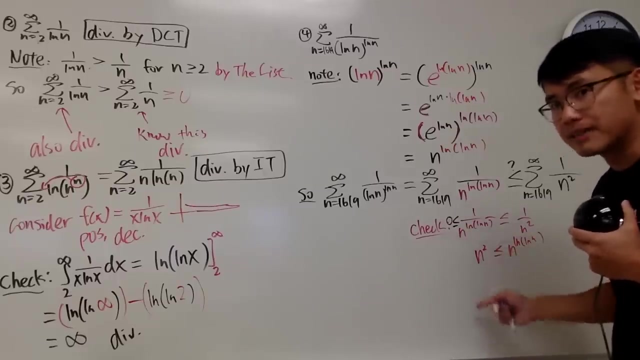 And notice that everybody is positive. okay, And then cross-multiply, you can just get n squared. Is this less than or equal to n? to the ln, n, ln, ln, n Like this? Well, the base they are the same, just n and n is positive. 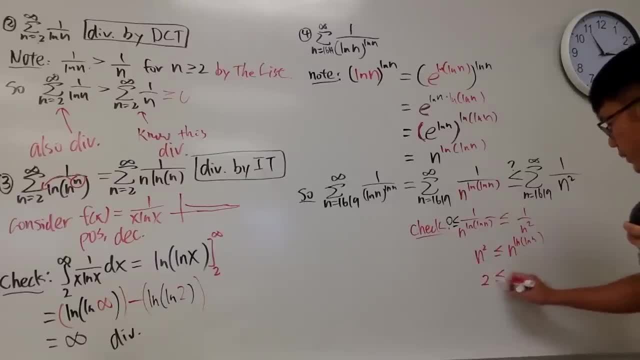 So you can just ignore the base. Compare the power: Is 2 less than or equal to? right here, I still don't know yet. Is 2 less than or equal to ln of ln, n, And what we care about is just 4.. n is. 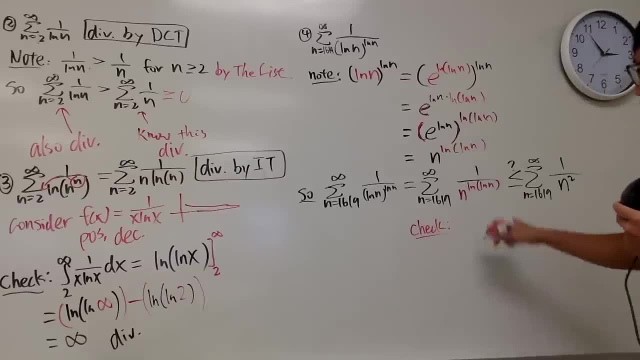 right here. So if you would like, you can do the check, which is well, we just have to check. 1 over n ln ln n power. Is this less than or equal to 1 over n squared? You can cross-multiply real quick. 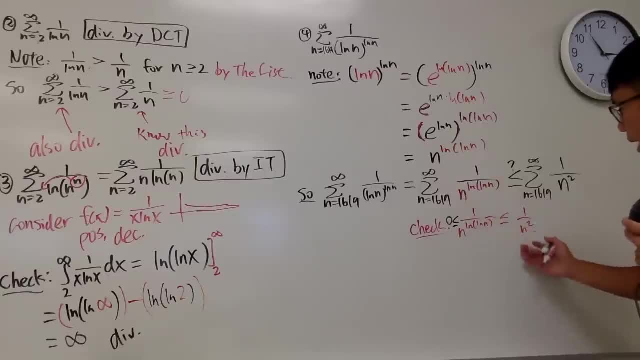 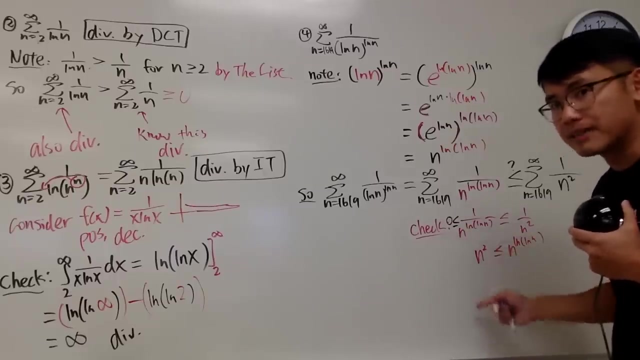 And notice that everybody is positive. okay, And then cross-multiply, you can just get n squared. Is this less than or equal to n? to the ln, n, ln, ln, n like this? Well, the base they are the same, just n and n is positive. 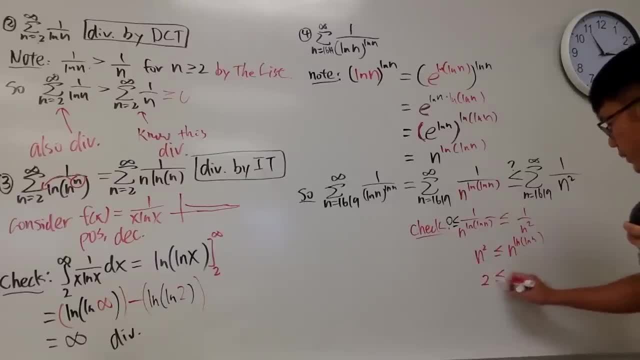 So you can just ignore the base. Compare the power: Is 2 less than or equal to? Right here, I still don't know yet. Is 2 less than or equal to ln of ln, n, And what we care about is just 4.. n is. 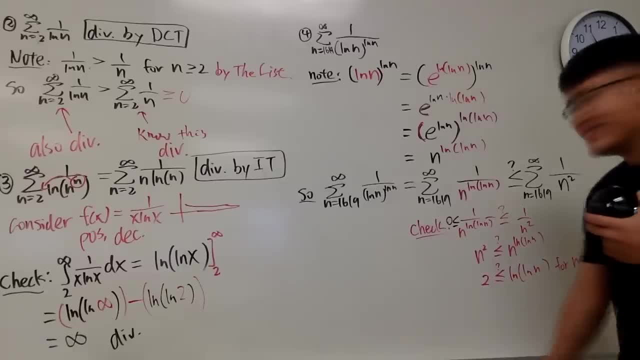 greater than or equal to 16, 19.. Well, this is pretty clear, because right here you know this is infinity, But the truth is you can keep going, right, You can keep going, And you can just do e to the second power. Is this less than or equal to? 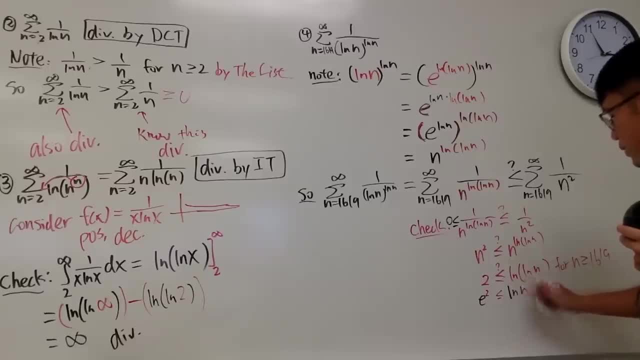 ln n, Because I do e to the power on both sides, And now I will just do it again, So I have e to the e squared. Is this less than or equal to n? And the truth is yes. this right here is actually about. 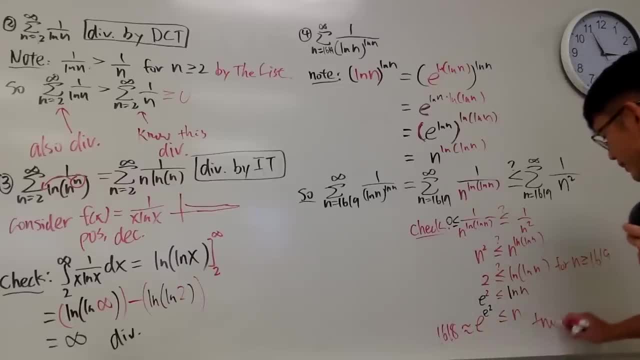 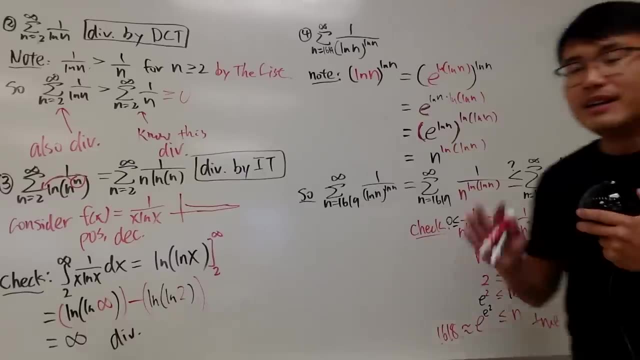 16, 18.. So this right here is actually true. n is bigger than 16, 18, because we care about. n is bigger than or equal to 16, 19.. The reason that I start with this big number is to make this work out. 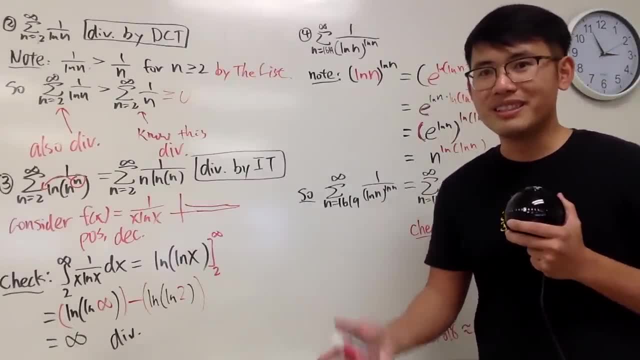 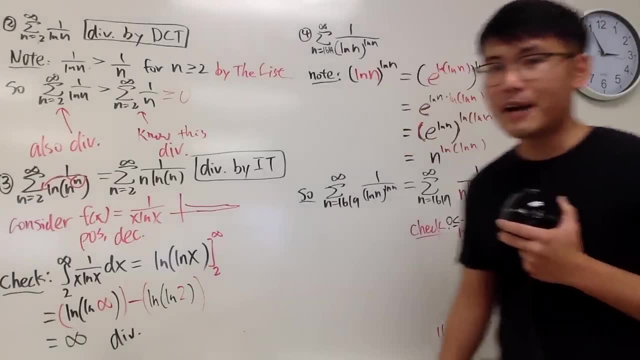 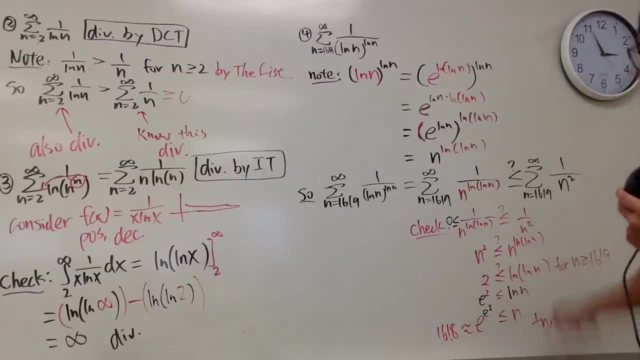 nicely, without any confusion about inequality. Especially, I know some students, for some students were just doing the series for the first time, So I don't want to cause any confusion, So I would just do this kind of things And of course, in fact, 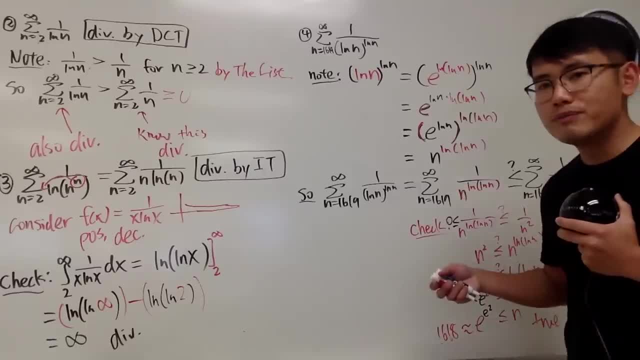 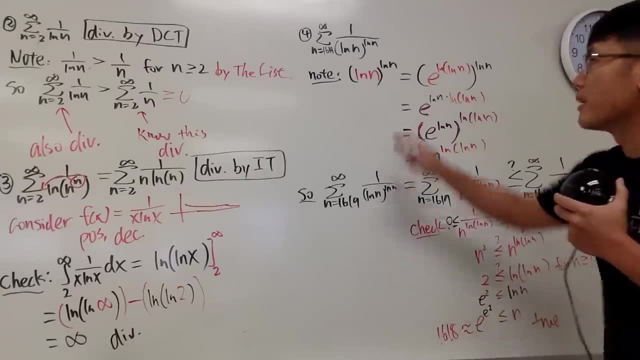 you can also use 1 over n to the third power or so, But in that case this number might not help And in that case I will actually give you guys a hint. I will say, hey, compare this with the sum. 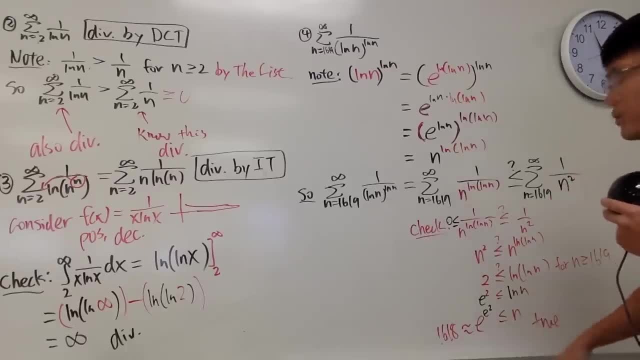 of 1 over n squared and just kind of work out the inequality. if this is true- And you know that, this right here and now let's just draw the arrows- We know that this, right here, converges because p is 2, which is: 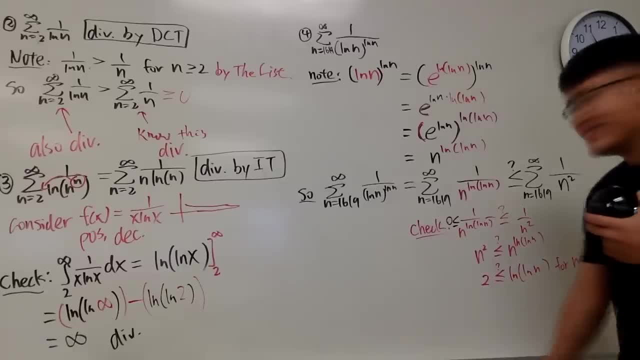 greater than or equal to 16, 19.. Well, this is pretty clear, because right here you know this is infinity, But the truth is you can keep going, right, You can keep going, And you can just do e to the second power. Is this less than or equal to? 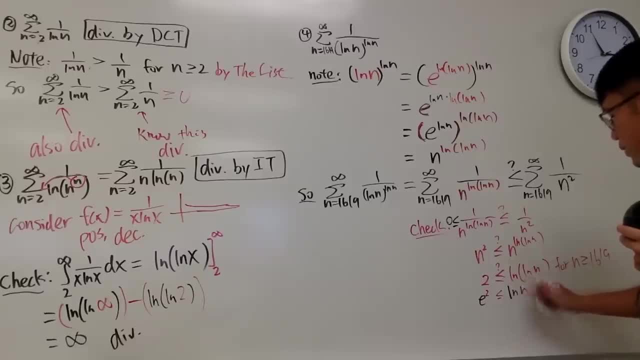 ln n, Because I do e to the power on both sides, and now I will just do it again, So I have e to the e squared. Is this less than or equal to n? And the truth is yes. this right here is actually about. 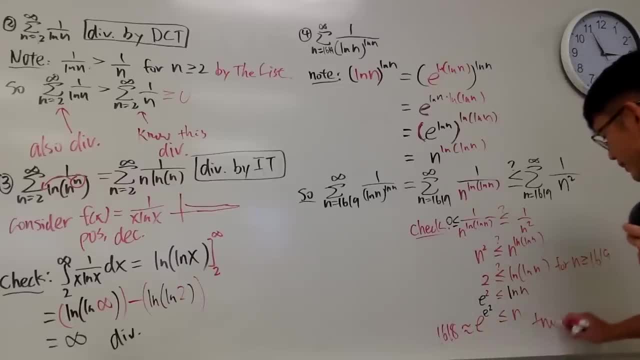 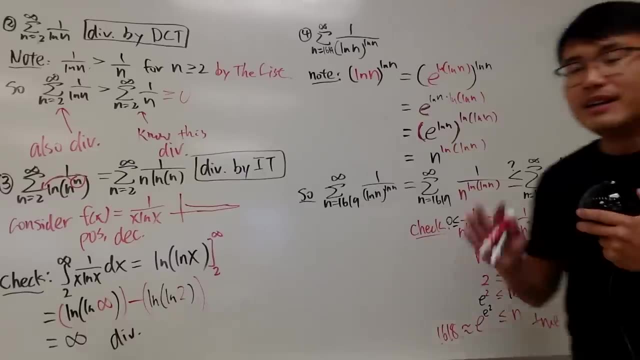 16, 18.. So this right here is actually true. n is bigger than 16, 18, because we care about. n is bigger than or equal to 16, 19.. The reason that I start with this big number is to make this work out. 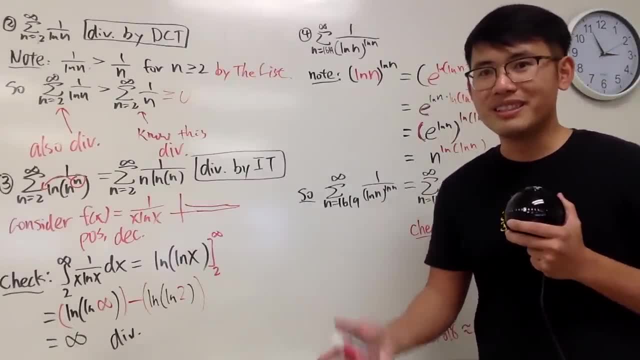 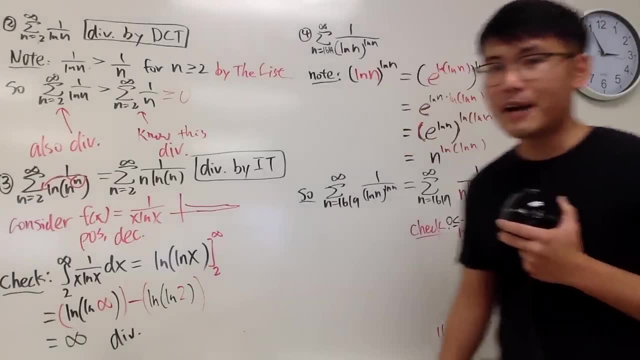 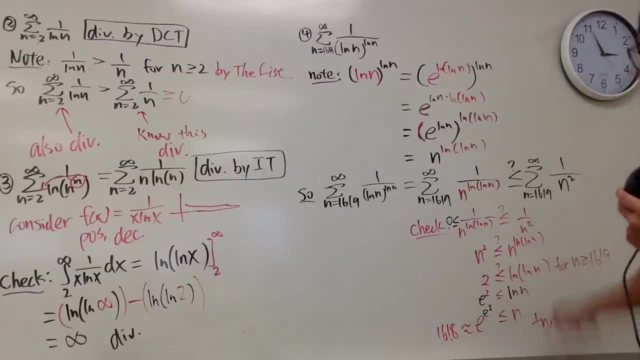 nicely, without any confusion about the inequality. Especially, I know some students, for some students were just doing the series for the first time, so I don't want to cause any confusion, So I would just do this kind of things And of course, in fact, 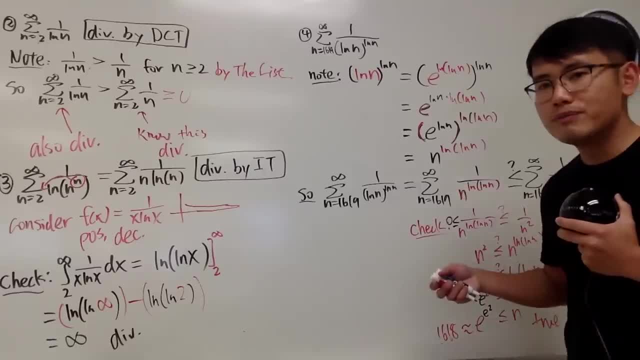 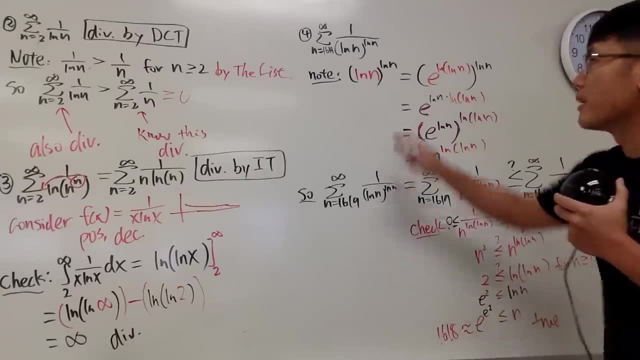 you can also use 1 over n to the third power or so, But in that case this number might not help, And in that case I will actually give you guys a hint. I will say: hey, compare this with the sum of. 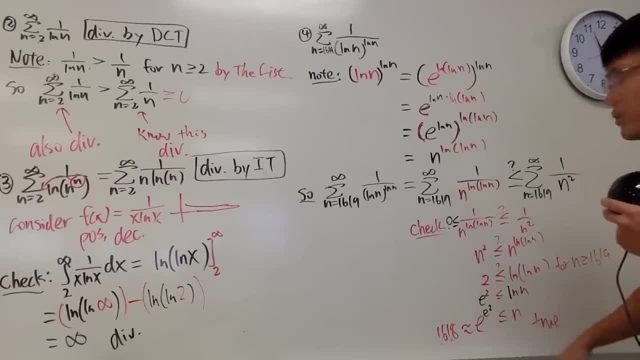 1 over n squared and just kind of work out the inequality. if this is true- And you know that this right here and now let's just draw the arrows- We know that this, right here, converges because p is 2, which is greater than 1.. 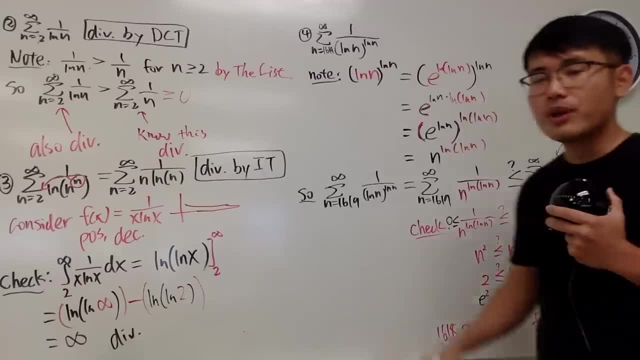 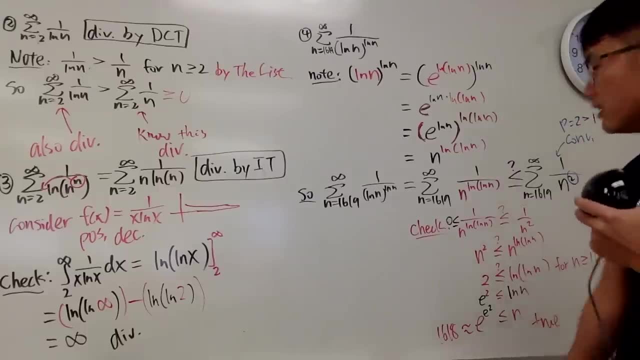 greater than 1.. Don't just put on p is 2.. You have to remember p is greater than 2 in order for the p-series to converge. This converge and the beauty is that this right here is smaller than the convergent. The idea is: if you have 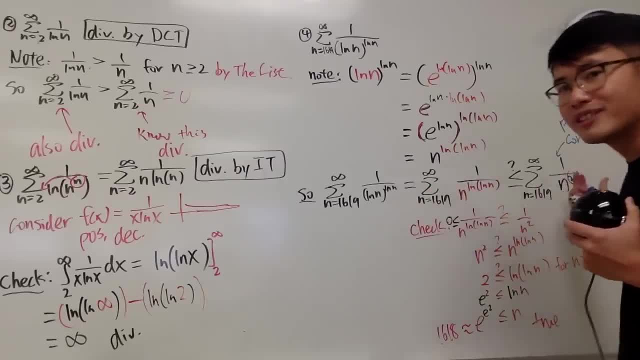 a young person. you can find somebody else who is younger than the young person. What can you say about this person? This right here is also young, but in series we call this convergent, So also converges. So that's the idea. 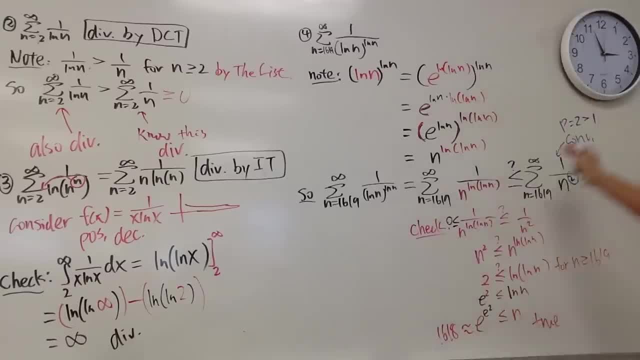 Don't just put down p is 2.. You have to remember p is greater than 2 in order for the p series to converge. This converge and the beauty is that this right here is smaller than a convergent. The idea is: if you have 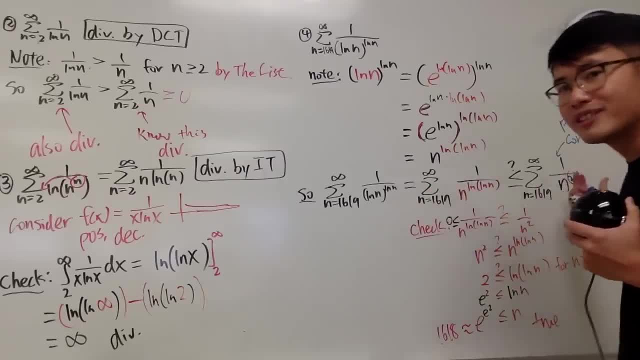 a young person. you can find somebody else who is younger than a young person. What can you say about this person? This right here is also young, but in series we call this convergent, So also converges. So that's the idea. 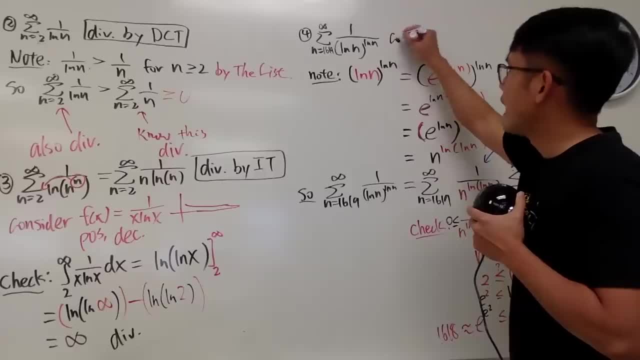 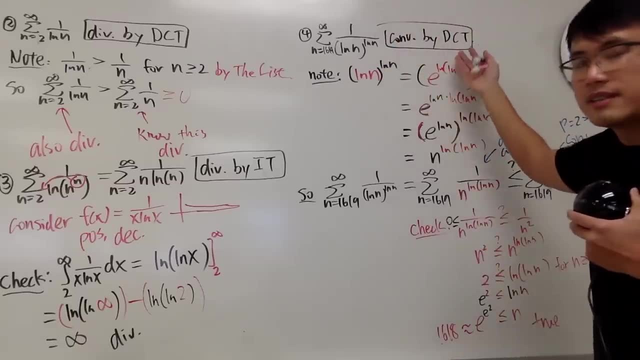 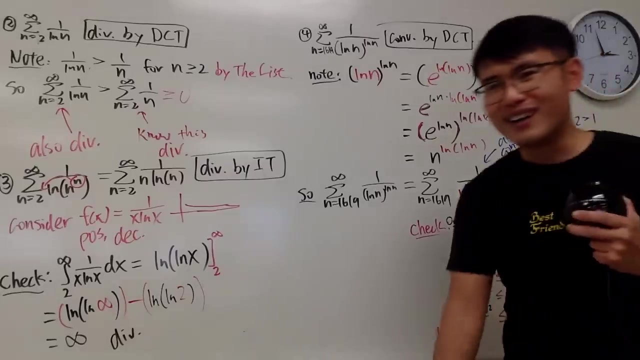 So we'll come back here and we'll say this right here: converges by direct comparison test, And the reason that we are saying direct comparison test is because we use the inequality. So that's the idea For number 4.. Right here. 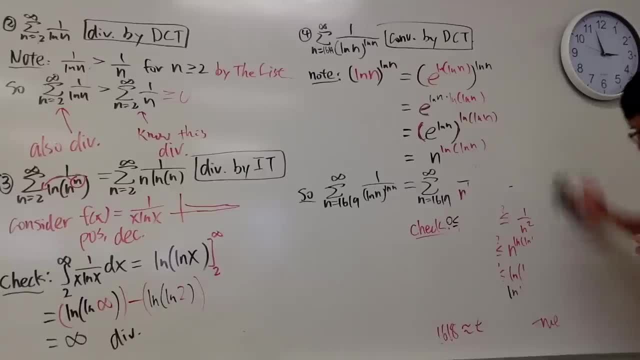 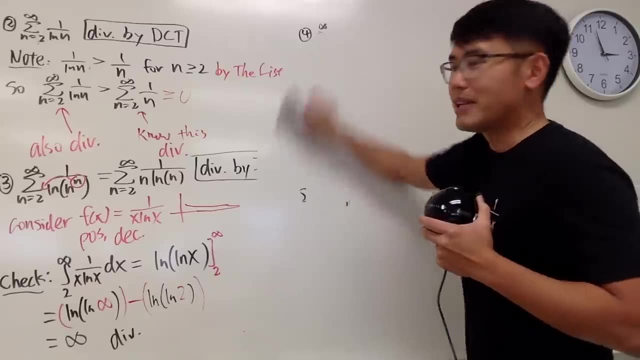 Take a look, take a look, take a look. Good, So again, whenever I'm erasing the board, I just like talk to you guys. So let me know what classes are you guys taking and, oh yeah, let me know how old you guys are as well. 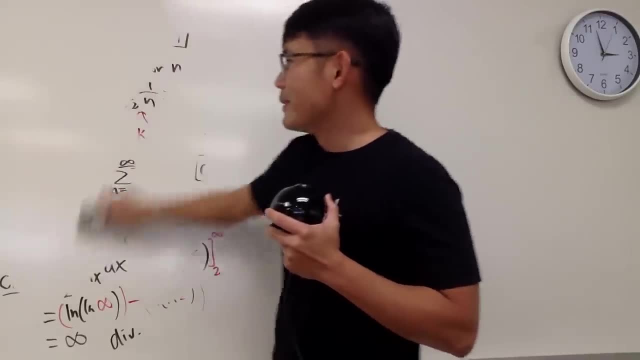 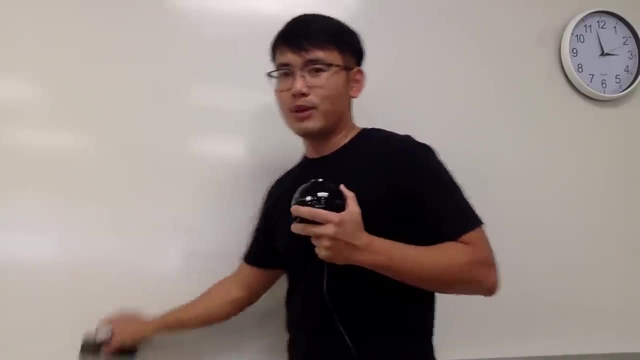 Because I know nowadays I have a lot of younger viewers. It's like amazing. I don't even know what I was doing when I was like 12 years old. Some people are like 12 years old and they're doing calculus already, In fact, 10.. I knew. 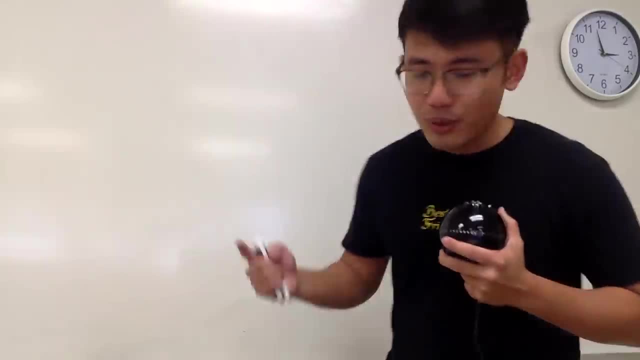 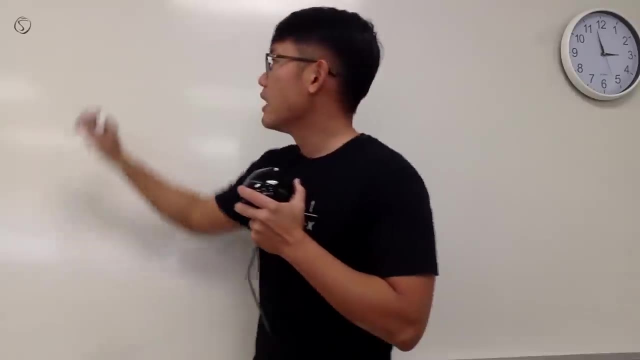 Wuhan, for example. Give you a shout out over there. Okay, continue Number 5.. Right here, This is the question. I will write it down right here for you guys. We are looking at the sum as n goes from 1 to infinity. 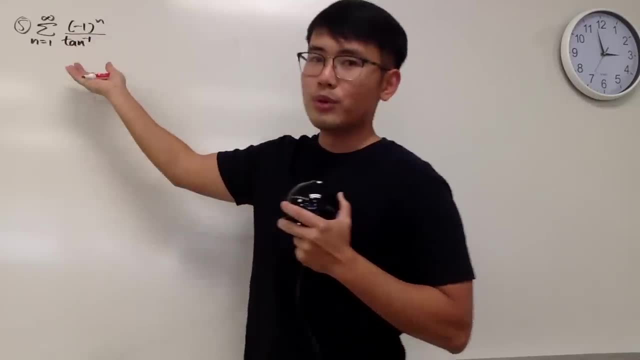 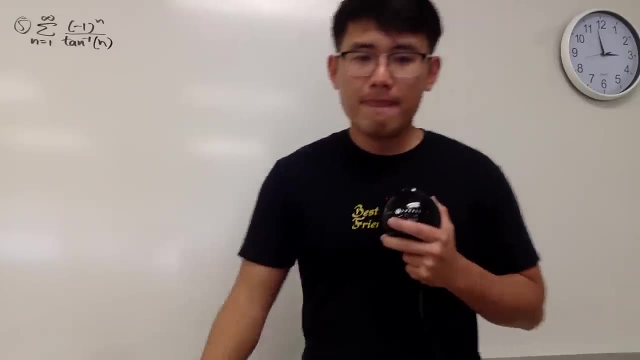 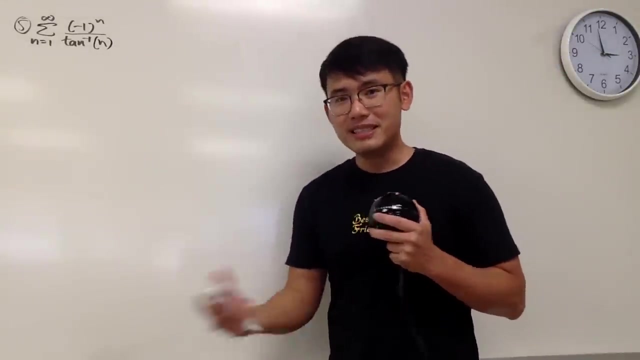 negative 1 to the nth power over the inverse tangent with this horrible notation that nobody likes. So n like that, right? So, hmm, Yeah, that's the question. So what do you guys think about that? Notice, Inverse tangent is not. 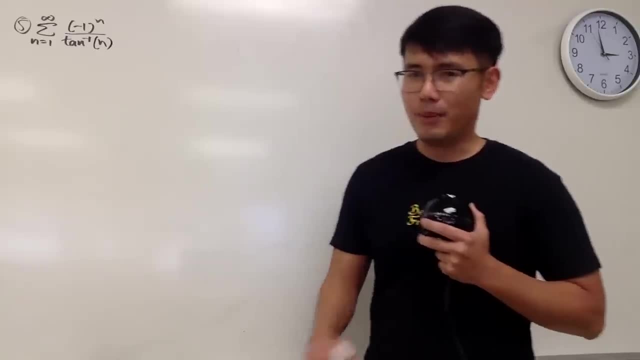 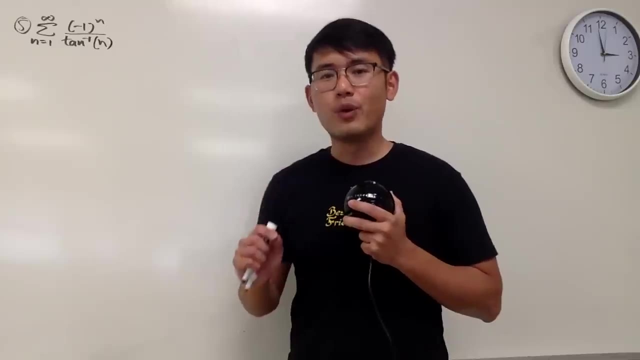 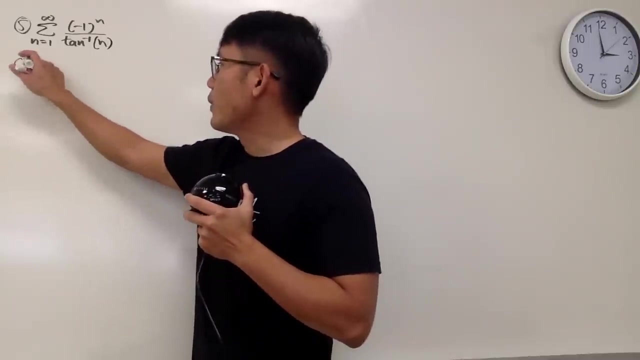 invited on the list because inverse tangent does not approach infinity. So the truth is this: right here we can do what we call the test for divergence And some books they also call it the limit test. So I will just show you guys this right here. So what we are going to do. 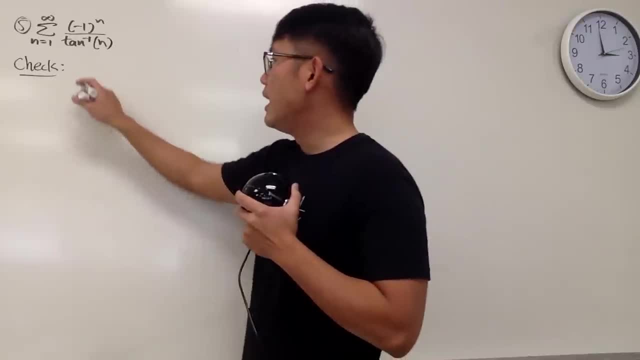 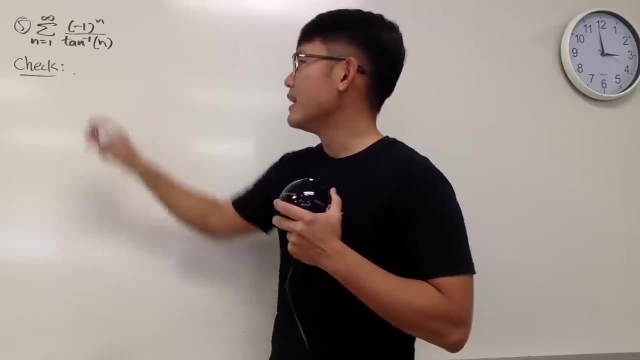 is: let's just go ahead and check the limit, And I will just write this down right here for you guys: Whenever we check the limit, I think I will just do this right. I will just say, as n goes to infinity like this: 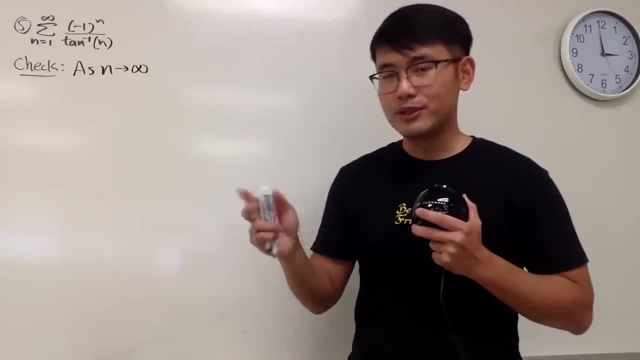 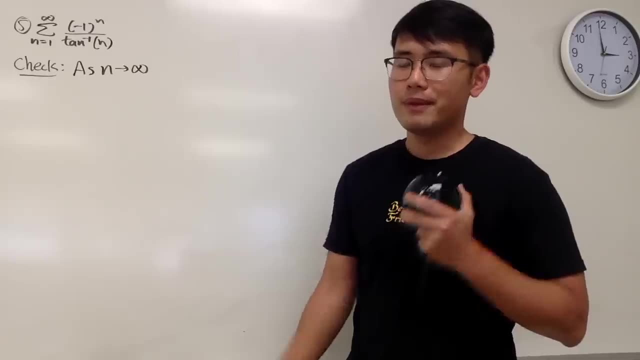 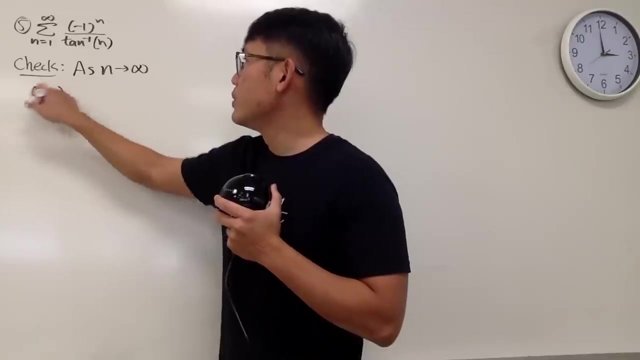 Because this way I don't have to write down the LIM so many times. And of course, these notations are interchangeable, so just depending on how you like it. Okay, here we go. Let's look at this. Which is negative one to the? 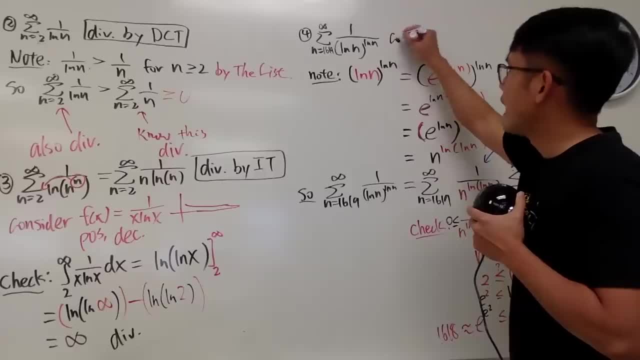 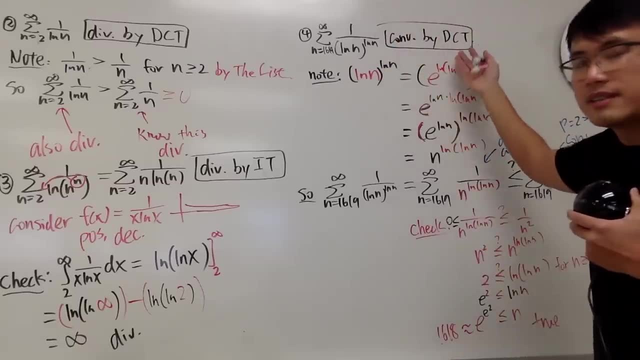 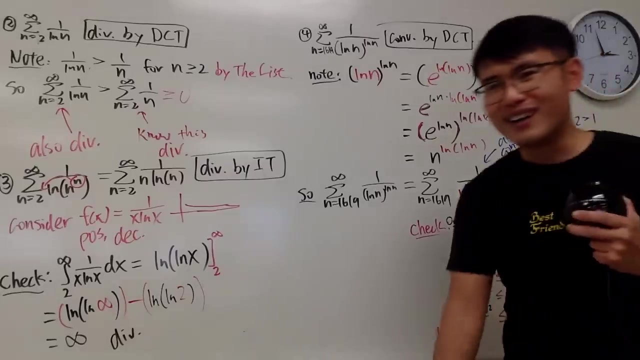 So we'll come back here and we'll say this right here: converges by direct comparison test, And the reason that we are saying direct comparison test is because we use the inequality. So that's the idea For number 4.. Right here. 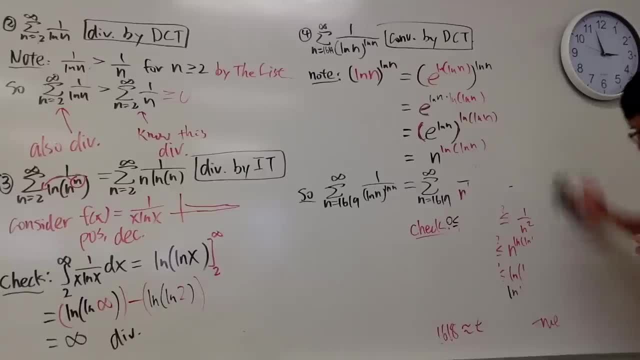 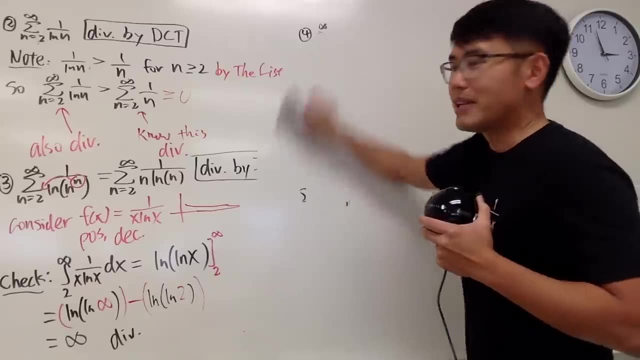 Take a look, take a look, take a look. Good. So again, whenever I'm erasing the board, I just talk to you guys. So let me know what classes are you guys taking and, oh yeah, let me know how old you guys are as well. 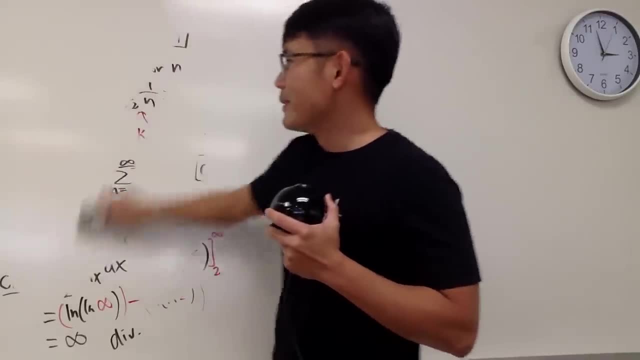 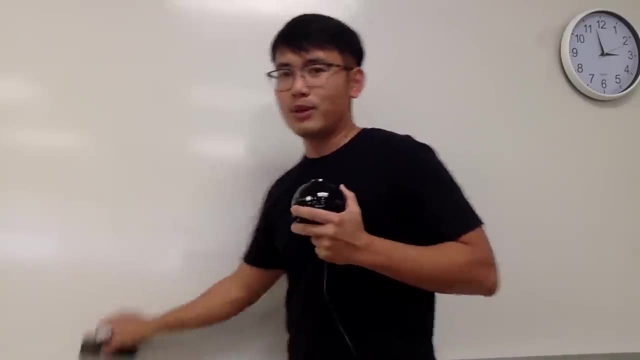 Because I know nowadays I have a lot of younger viewers And it's like amazing. I don't even know what I was doing when I was like 12 years old. Some people are like 12 years old and they're doing calculus already, In fact, 10.. 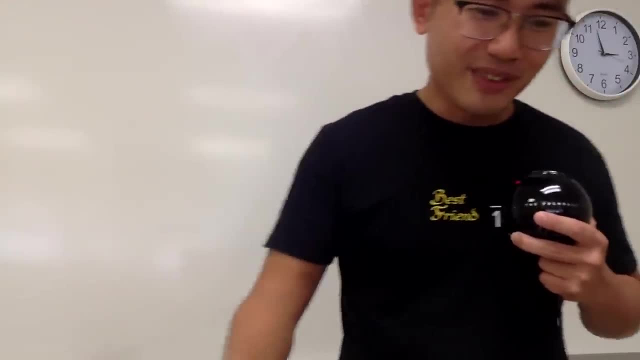 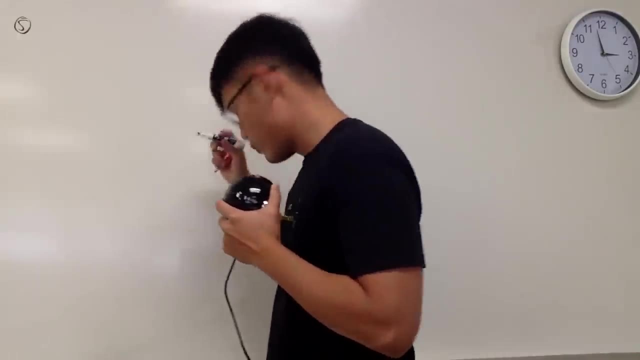 I knew Wuhan, for example. I'll give you a shout out over there. Okay, continue Number 5.. Right here, This is the question. I will write it down right here for you guys. We are looking at the sum as n goes from 1 to. 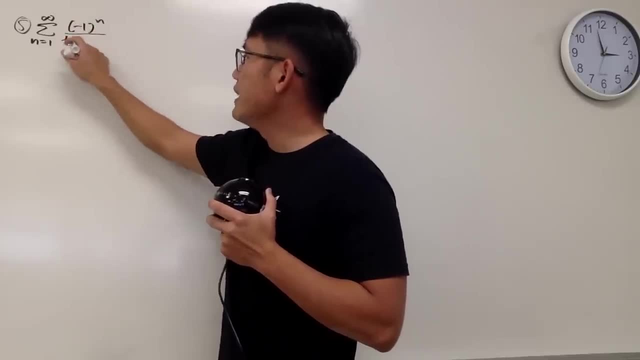 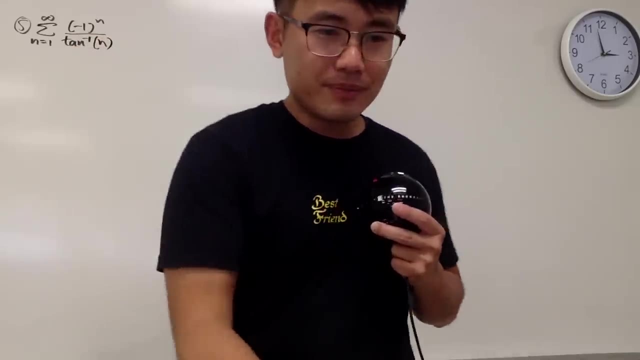 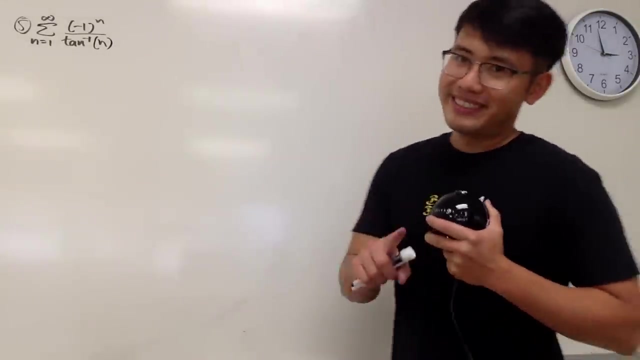 infinity negative 1 to the nth power over the inverse tangent, with this horrible notation that nobody likes Of n, like that, right? So, hmm, Yeah, that's the question. So what do you guys think about that? Notice, inverse tangent is not. 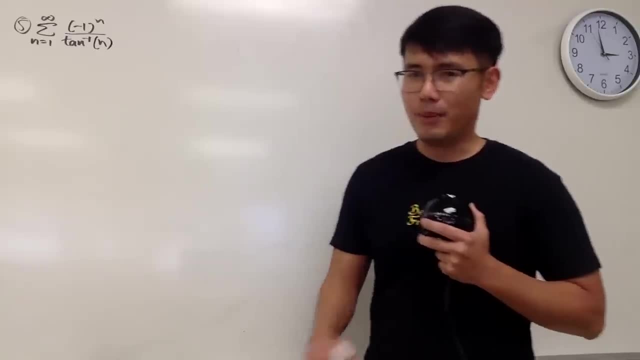 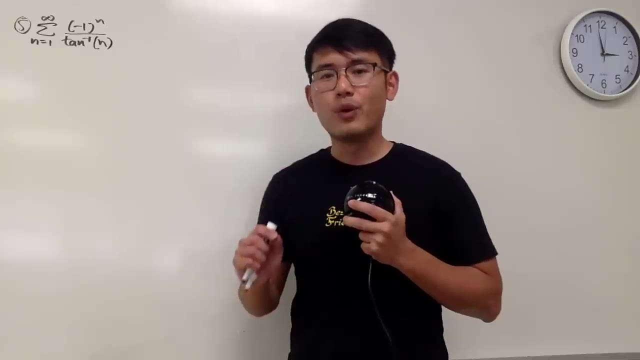 invited on the list because inverse tangent does not approach infinity. So the truth is this: right here we can do what we call the test for divergence, And some books they also call it the limit test. So I'll just show you guys. 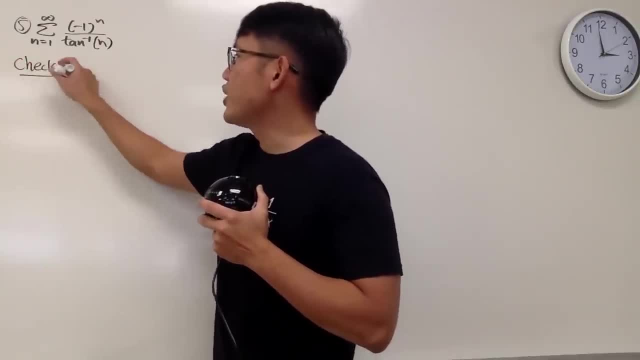 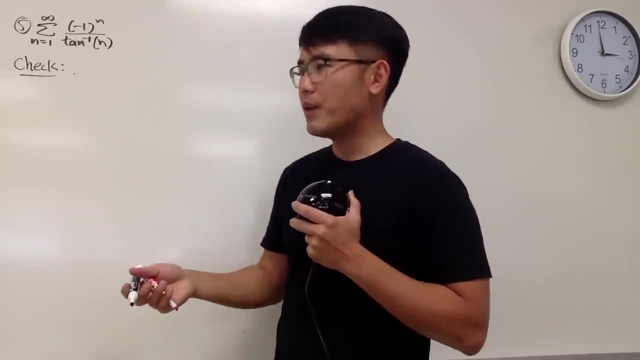 this right here. So what we are going to do is: let's just go ahead and check the limit, And I will just write this down right here for you guys: Whenever we check the limit, I think I will just do this right. I'll just say: 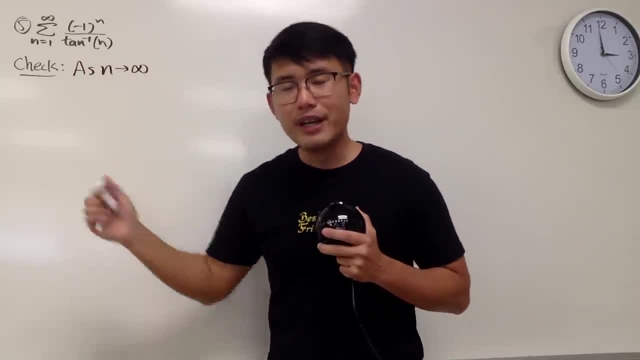 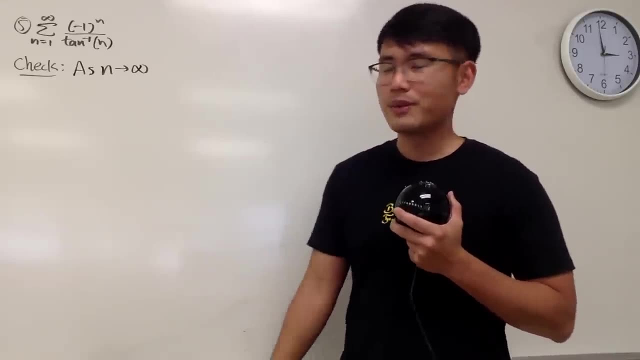 as n goes to infinity, like this, Because this way I don't have to write down the LIM so many times, And of course these notations are interchangeable. so just depending on how do you like it, I'll see. Okay, here we go. 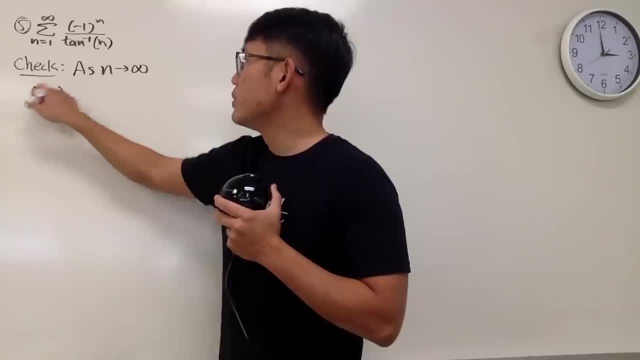 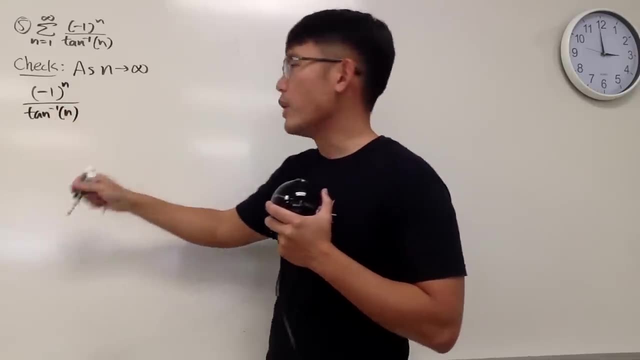 Let's look at this, which is negative: 1 to the nth power, over the inverse tangent of n, As n goes to infinity. well, this, right here I'll draw the arrow because we are taking the limit, meaning I'm putting infinity down here. 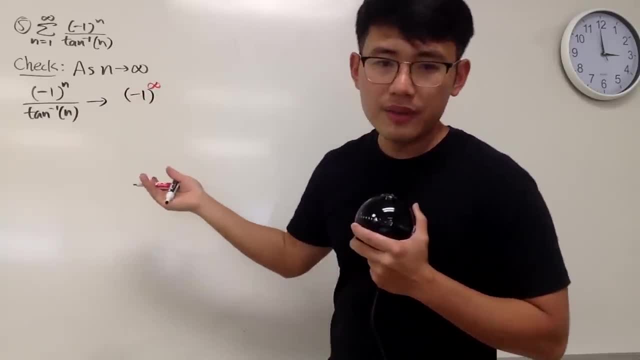 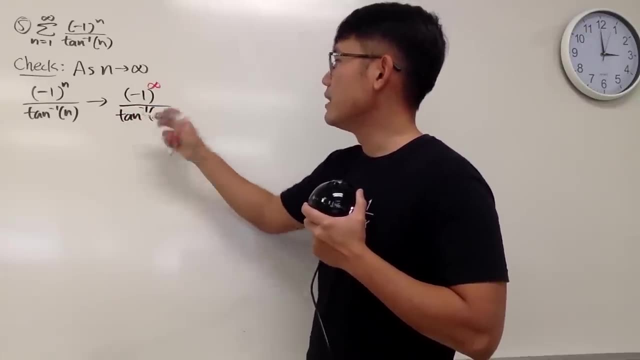 So it looks like we have negative 1, and on the top we have the little infinity symbol Over and here we have the inverse tangent of infinity, Like that. And check this out: This right here is actually what Pi over 2,. 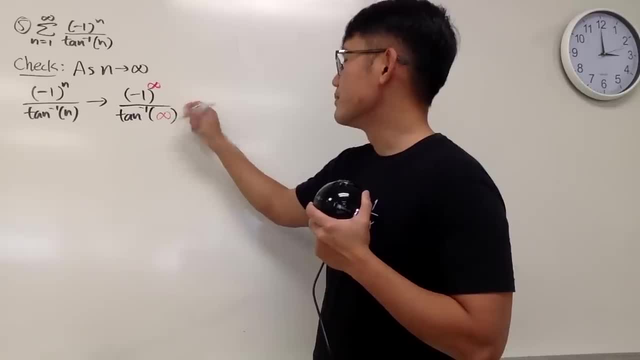 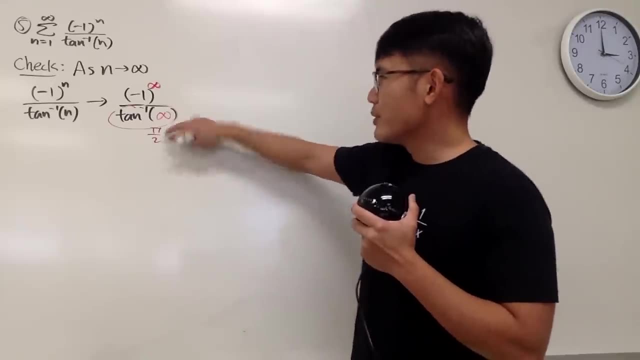 isn't it? So this right here is well depends on how you know. just put it down here. This is just pi over 2. And of course you can do more. you can put the 2 on the top and the pi on the bottom. 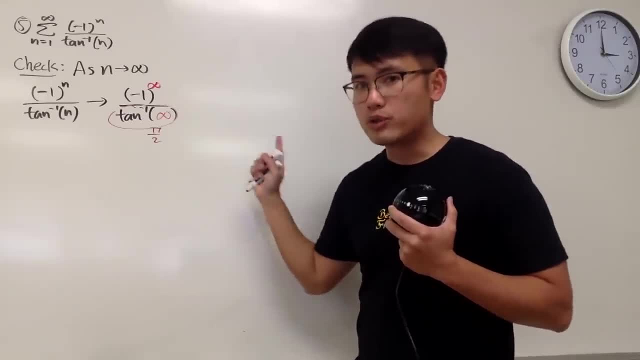 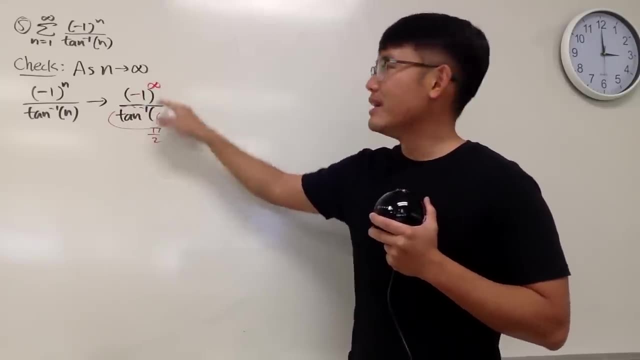 but the problem is that this right here does not approach 0. Even though you have like a trouble thing on the top negative 1 to the infinity, which is a really bad notation, the truth is this right here does not converge, This right here. 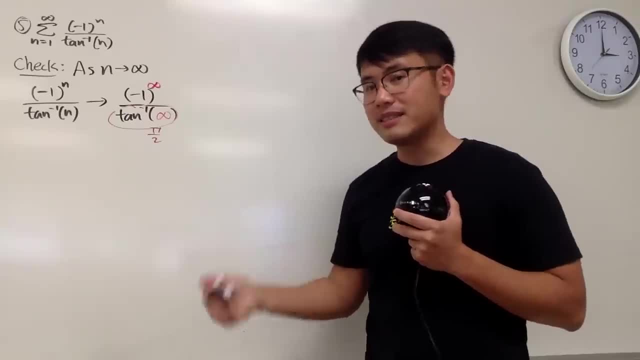 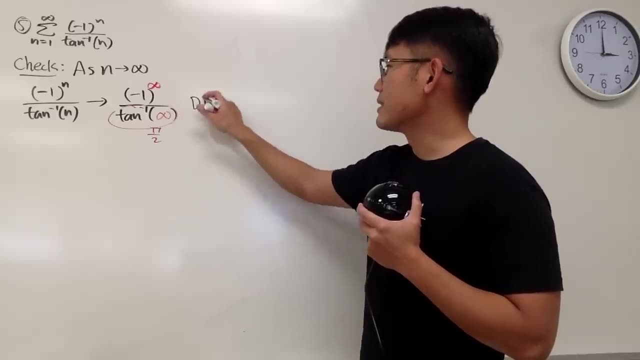 uniquely. it has no limit. the limit does not exist. I should have said that. So I'll just put down. this right here Does not exist, right, And I don't know why. sometimes I put down does not exist, I put down the dots and then the. 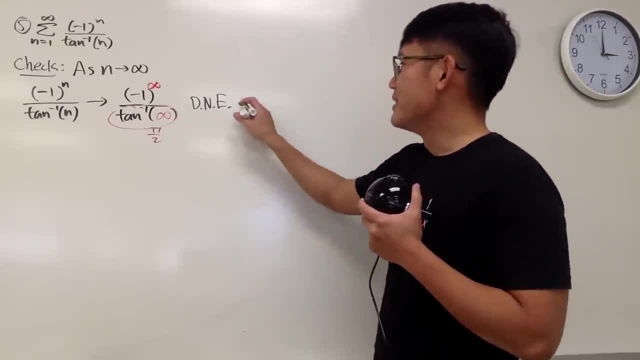 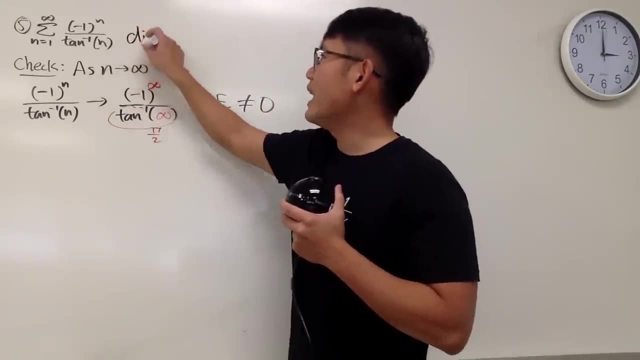 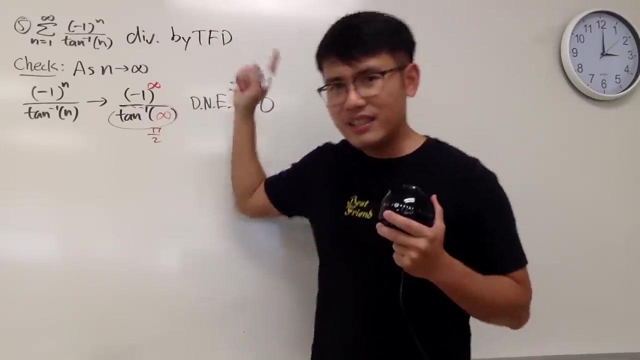 direct computer syntax. I don't put down dots, I don't know why. Does not exist, does not equal to 0. So what we can say is this: right here, diverges by the test for divergence, tfd. So cool. 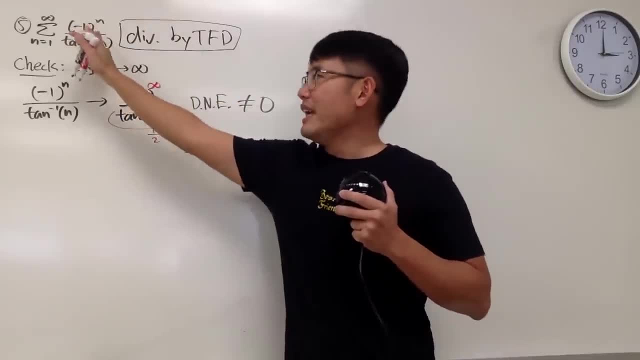 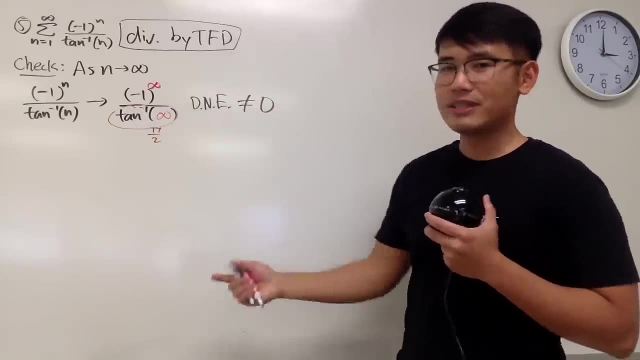 As long as you show the limit of the an is not equal to 0, as n goes to infinity, you are good to go Diverges, So that's what I said earlier. But if the limit of this does approach 0, we will have. 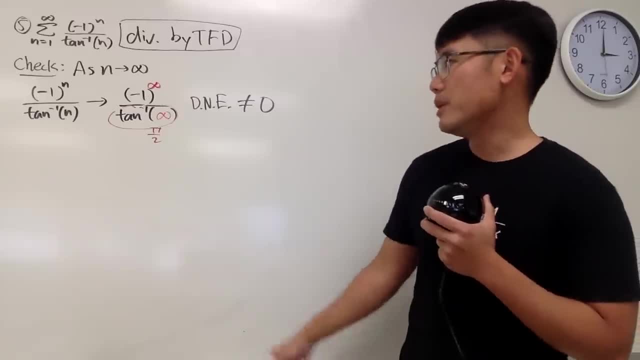 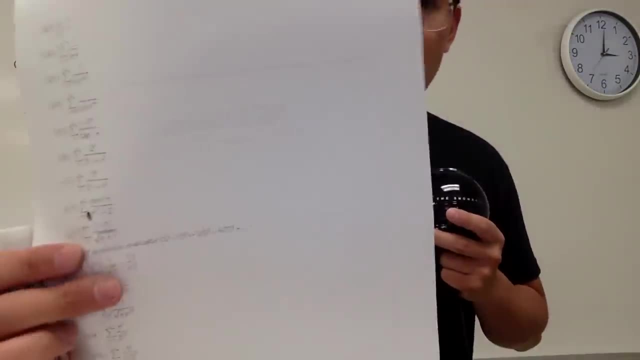 to do more work for that, unfortunately. Well, maybe we're lucky so we can do more calculus. So that's it Now. number six: Right here we have some powers Now, not power series, yet I will have some power. 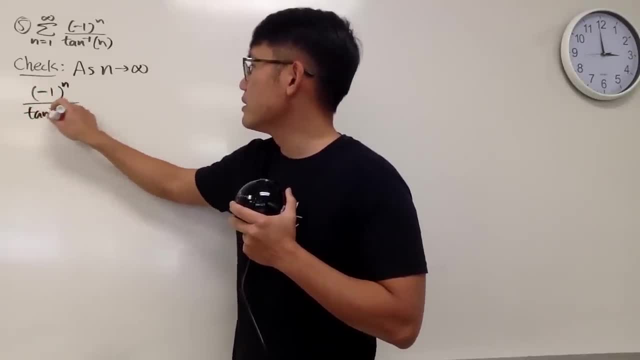 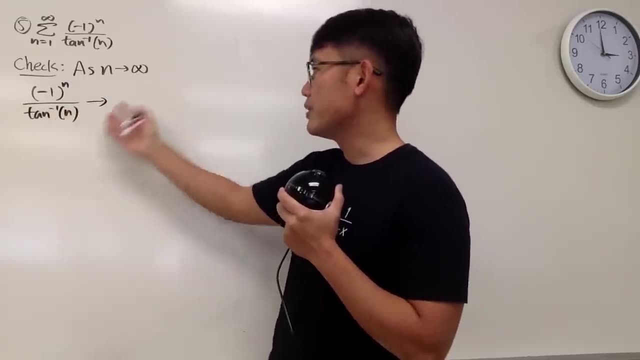 nth power over the inverse tangent of n, As n goes to infinity. well, this, right here I will draw an arrow, because we are taking a limit, meaning I am putting infinity down here, So it looks like we have negative one. and on the, 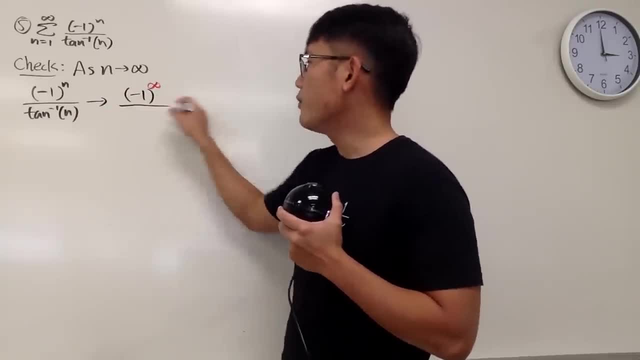 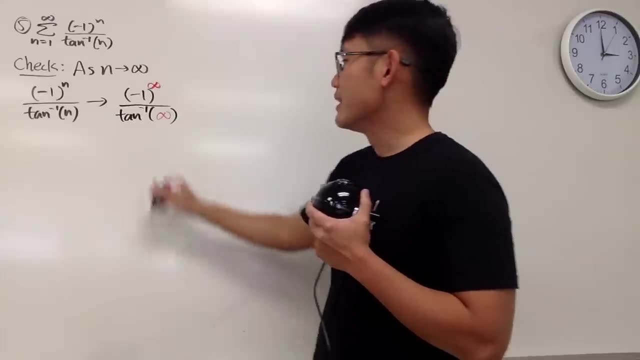 top we have the little infinity symbol Over and here we have the inverse tangent of infinity, Like that. And check this out: This right here is actually what Pi over two, Isn't it? So this right here is well. 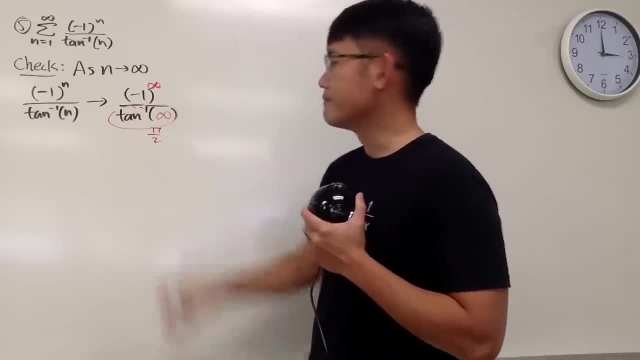 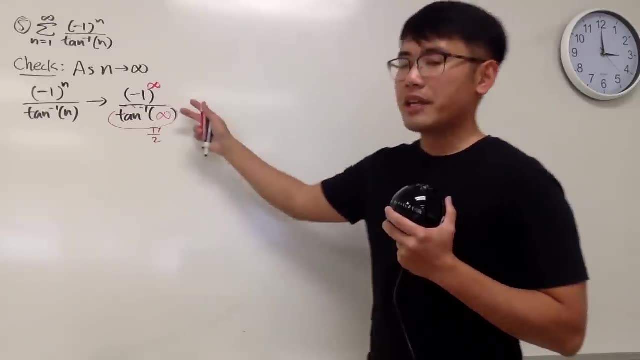 depends on how you know. just put it down here. This is just pi over two, And of course you can do more. You can put the two on the top and the pi on the bottom, But the problem is that this right here does not approach zero. 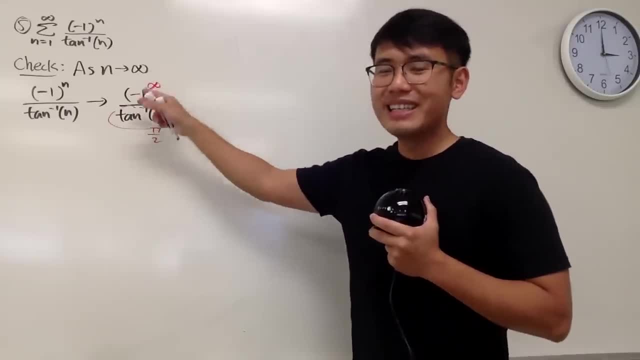 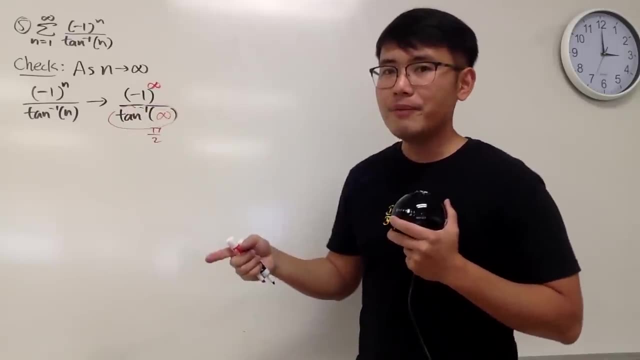 Even though you have like a trouble thing on the top, Negative one to the infinity, which is a really bad notation, The truth is, this right here does not converge, This right here. technically it has no limit, The limit does not exist. 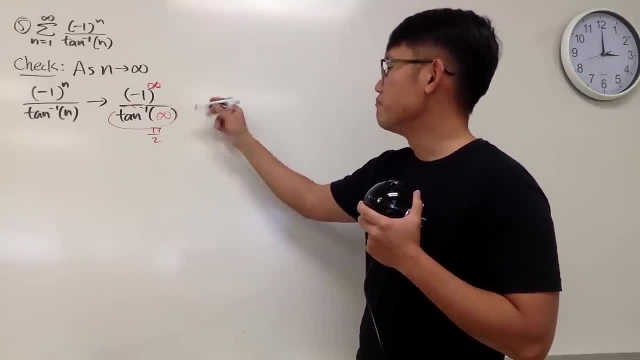 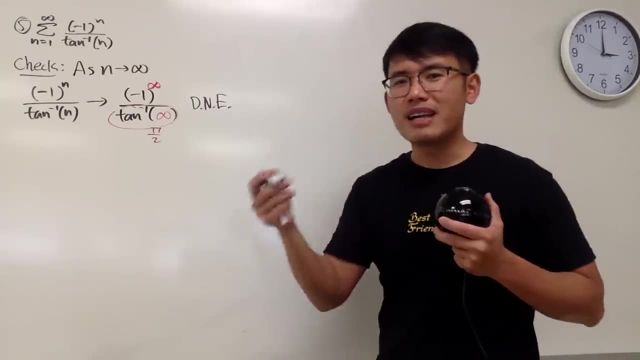 Actually I'll have to say that, So I'll just put down this right here Does not exist Right And I don't know why. sometimes I put down does not exist. I put down the dots And then the direct computation test. I don't put down dots, I don't know why. 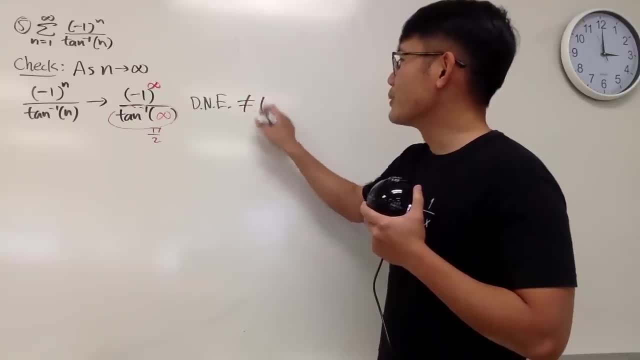 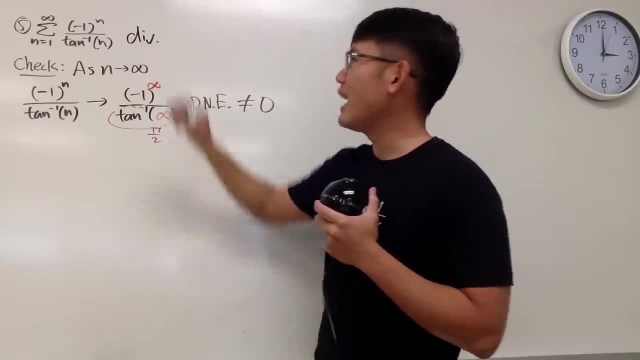 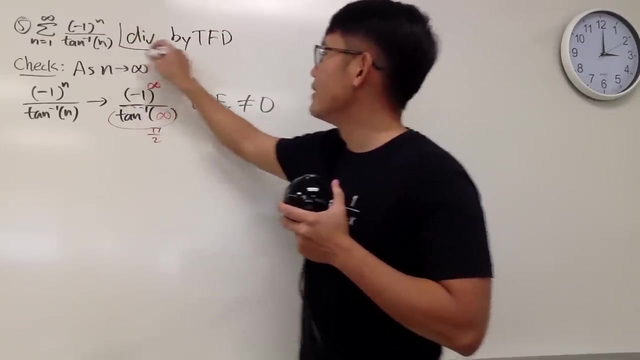 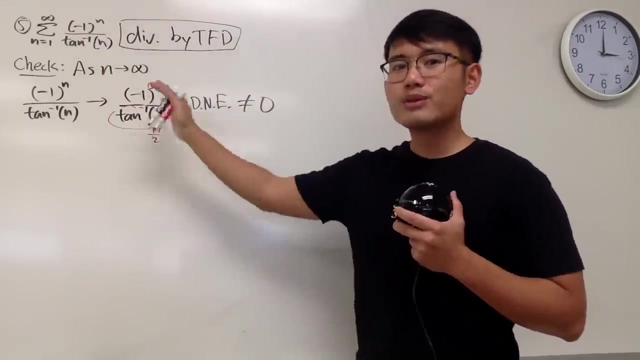 Does not exist, does not equal to zero. So what we can say is this: right here: diverges by the test for divergence tfd. So cool, As long as you show the limit of the an is not equal to zero, as n goes to infinity, you are. 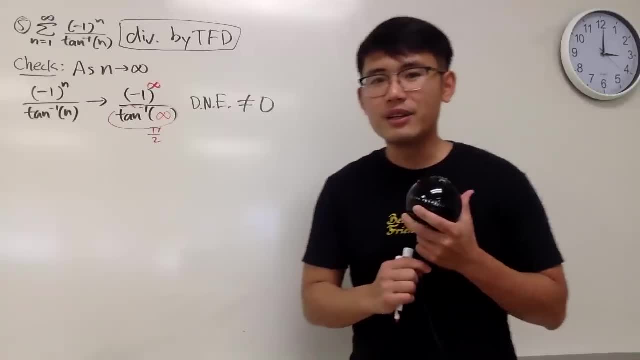 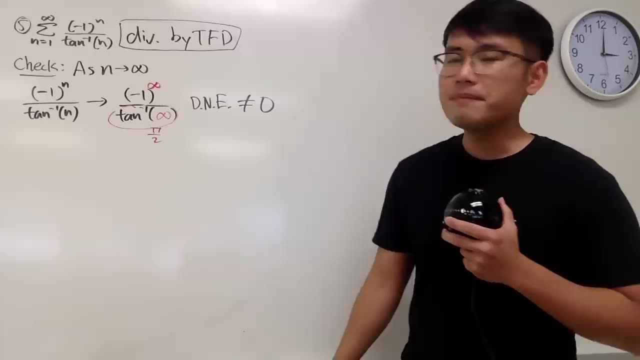 good to go. Diverges, Right. So that's why I said earlier, But if the limit of this does approach zero, we will have to do more work for that, unfortunately, Right? Well, maybe we're lucky so we can do more calculus. 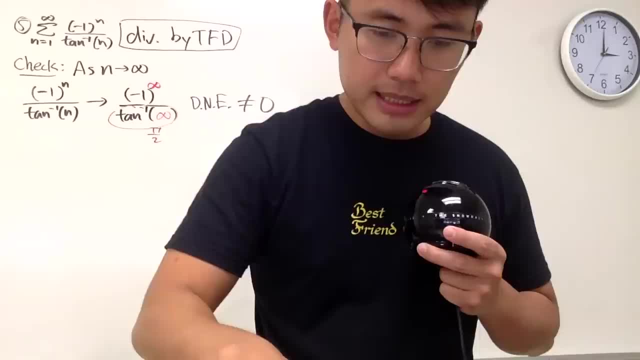 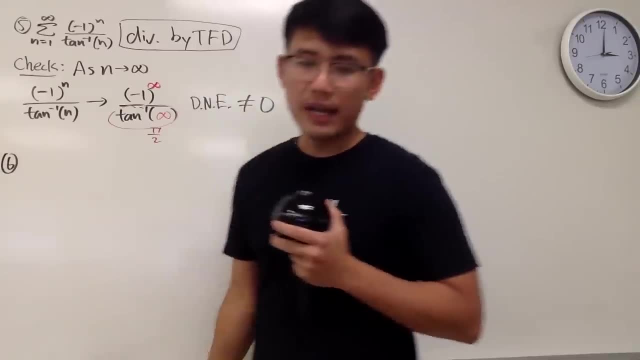 So that's it Now. number six: right here we have some powers now, Not power series, yet I will have some power series for you guys, Of course, the best friends, also in the video, of course. Okay, How can I make a? 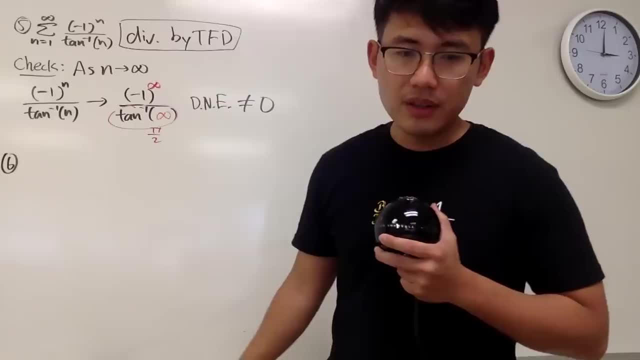 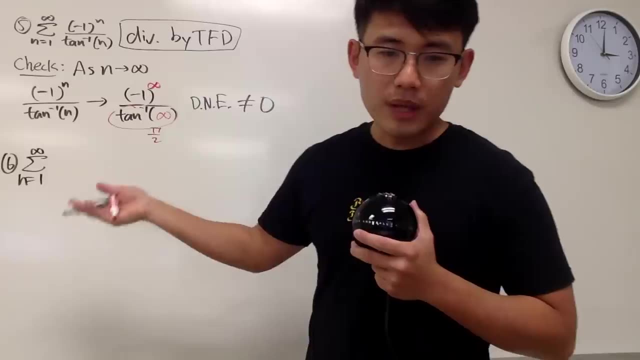 series for you guys. Of course, the best friends also in the video, of course. Okay, How can I make a video of series without mentioning the best friend, Right? So the limit as n goes from 1 to infinity, 2 to the nth power over. 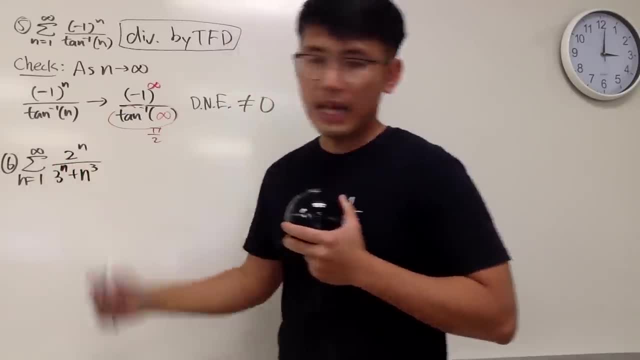 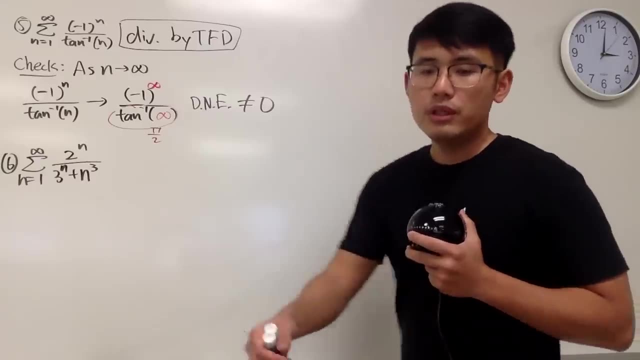 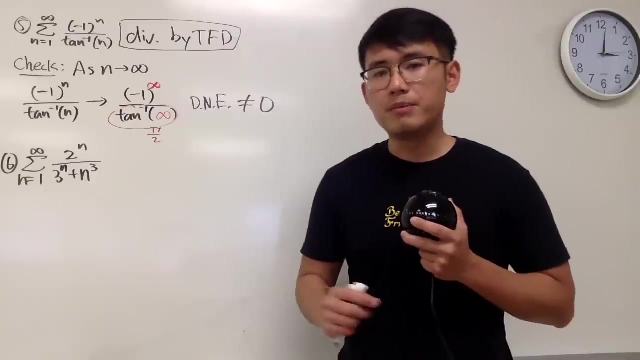 3 to the n plus n, cubed like this, Hmm, First of all, let's talk about the dominating part, which is, you know, just like you refer back to the list. When you have the list, you really can pick out the dominating part very. 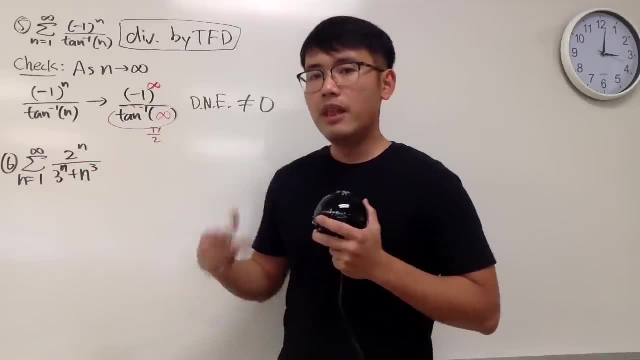 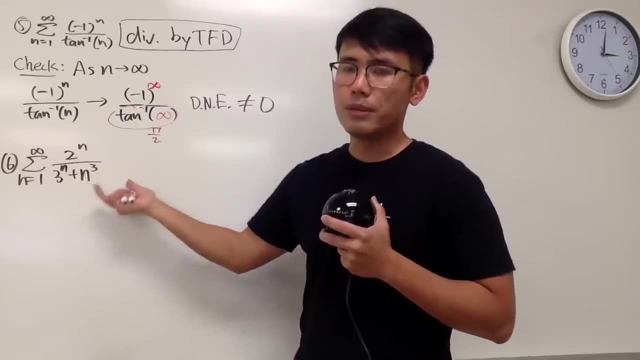 easily. Here we have 2 to the n, 3 to the n. they are the exponential part In another word, b to the n from the list, And this is n to a power, n to a third power, so n to the p right, We know. 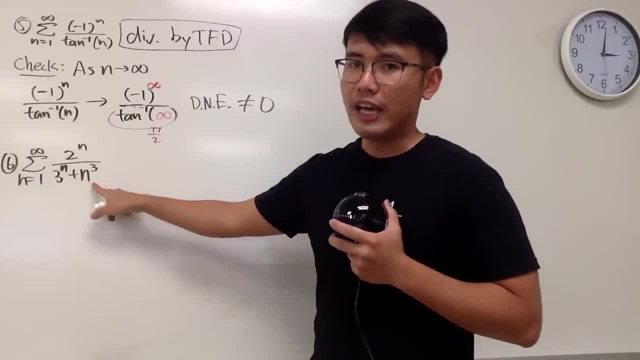 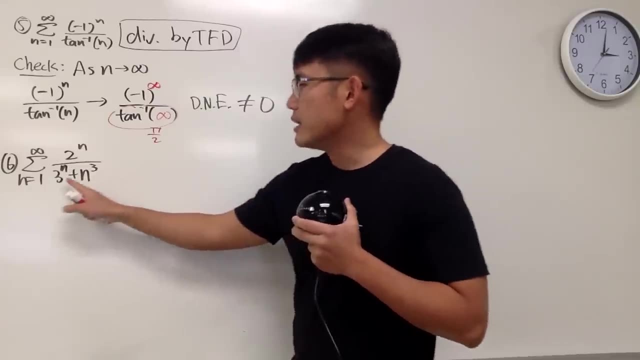 this will be bigger than that, so this guy has no say compared to that. In another word, we can kind of just cover that up. Okay, And now check this out. The truth is, everybody is positive. we're adding n to the third power right here. 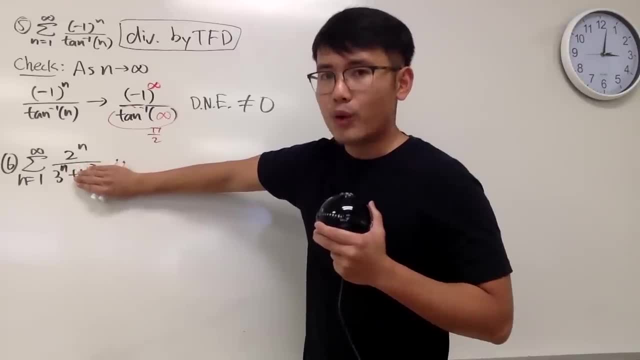 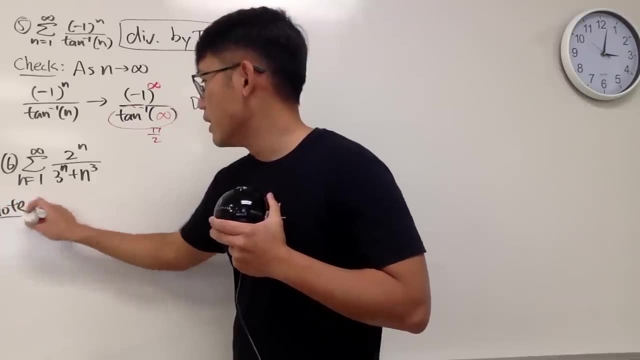 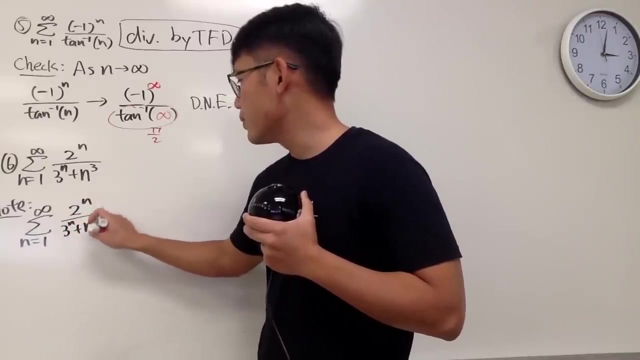 If you ignore the n to the third power, we can come with an inequality right away. We can say that: notice the sum as n goes from 1 to infinity, of 2 to the n over, 3 to the n plus n to the third power. 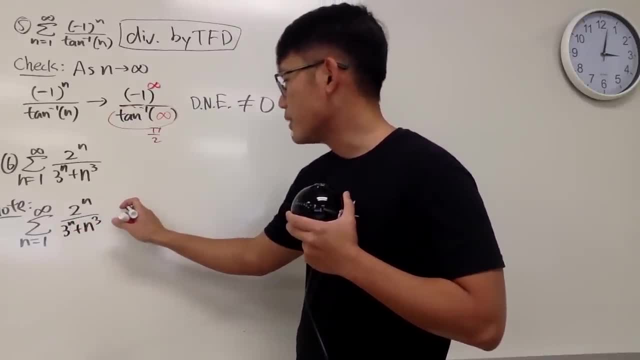 Let's just get rid of that. So in another word, we actually end up with less than well, technically you can also put on less than or equal to. I think I will just put on less than or equal to, all the way right. 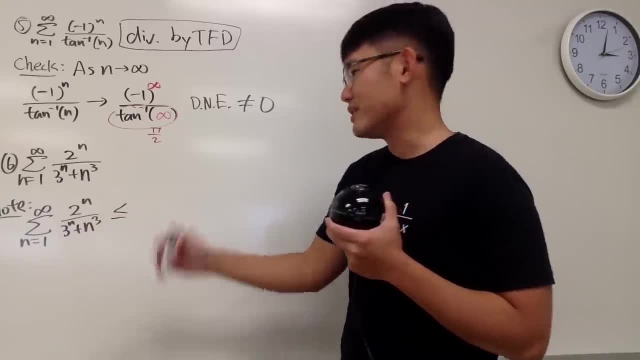 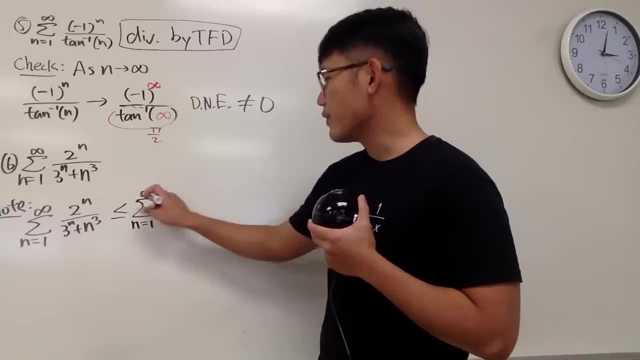 When you're comparing, just put on less than or equal to. I think that's how it goes. Anyway, get rid of that and we can say: this is the sum as n goes from 1 to infinity, which is 2 to. 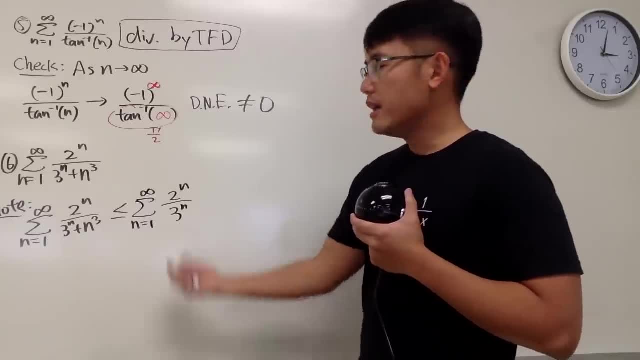 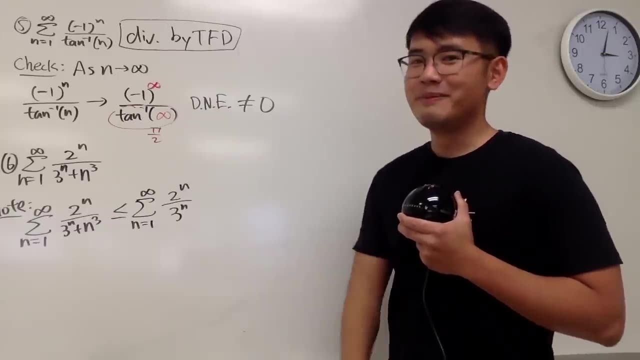 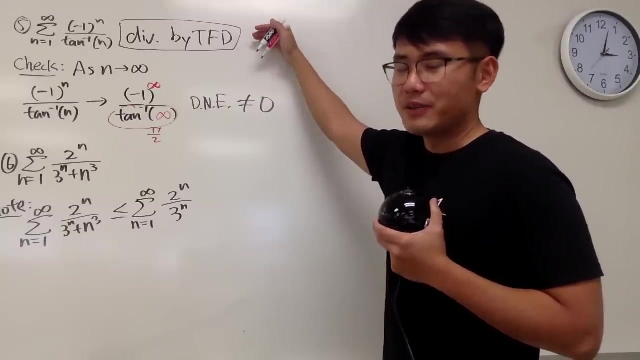 the nth power over 3 to the nth power, like that. This guy is bigger than that. this guy is less than that. This is not hard because it's easy. Please do not say this right here. diverges because it does not converge. 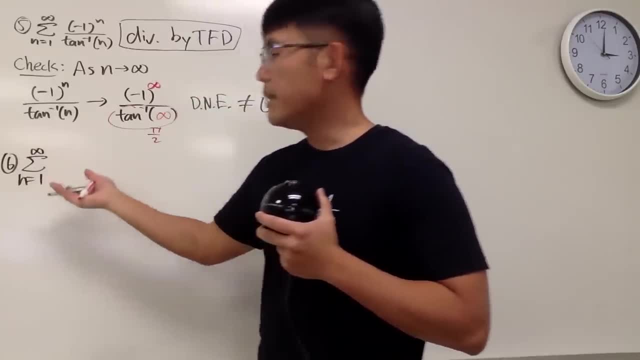 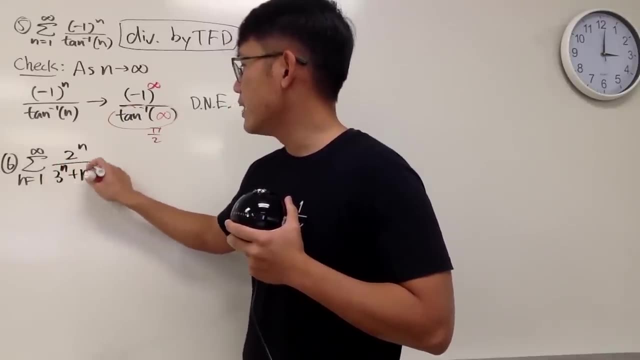 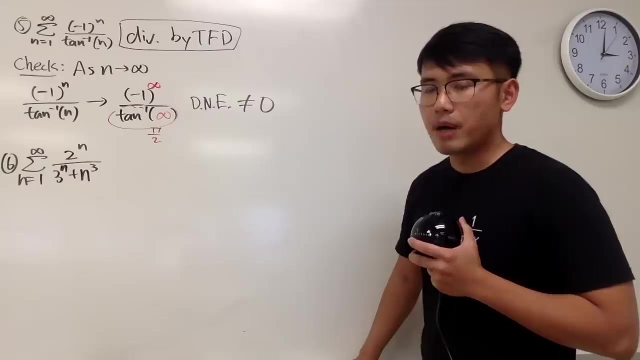 video of series, without mentioning the best friend Right. So the limit as n goes from one to infinity, two to the nth power, over three to the n, plus n cubed like this. Hmm, First of all, let's talk about the dominating part. 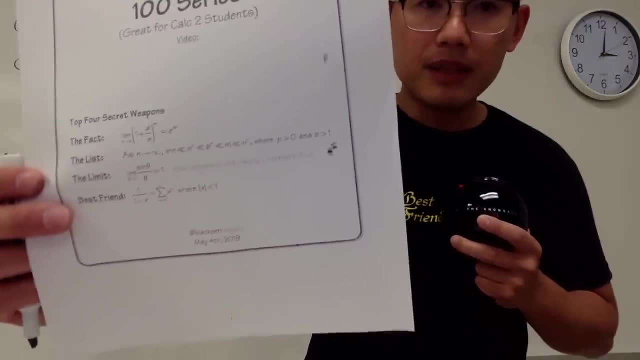 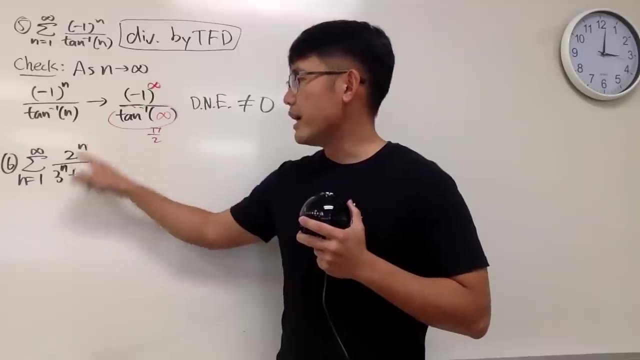 Which is you know. just like you refer back to the list. When you have the list you really can pick out the dominating part very easily. Here we have two to the n, three to the n. They are the exponential part, In another word. 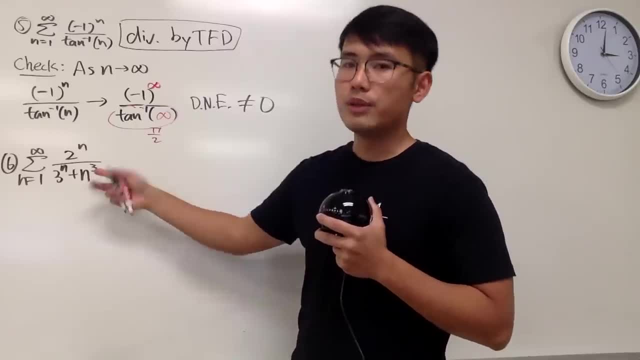 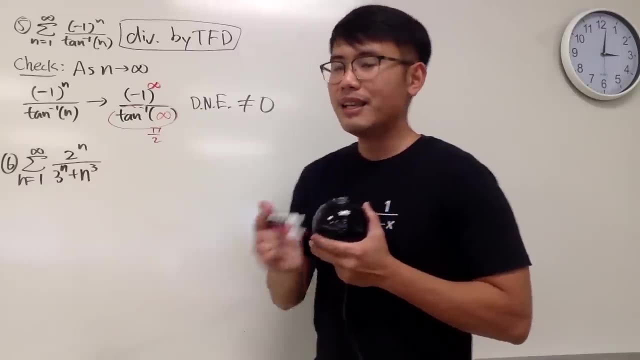 b to the n from the list, And this is n to a power, n to a third power, So n to the p right. We know this will be bigger than that, So this guy has no say compared to that. In another word, we can kind of 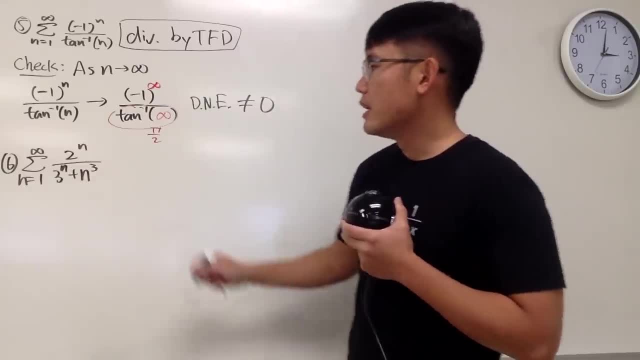 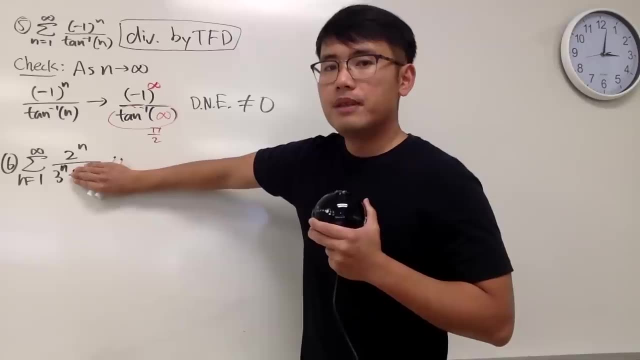 just cover that up, Okay, And now check this out. The truth is, everybody is positive. We're adding n to the third power right here. If you ignore the n to the third power, we can come with an inequality right away. 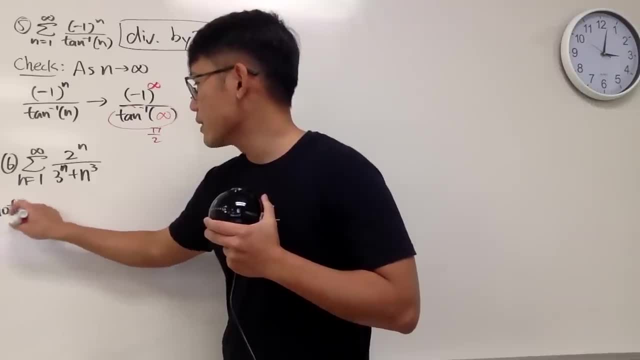 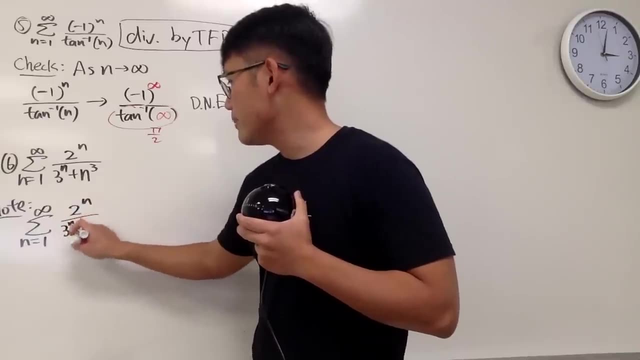 We can say that: notice the sum, as n goes from one to infinity, of two to the n over three to the n plus n to the third power. Let's just get rid of that. So, in another word, we actually end up with 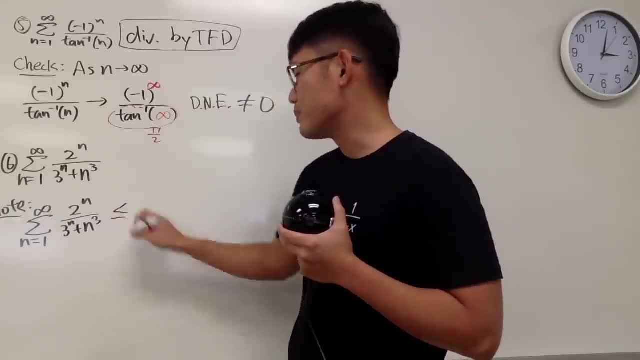 less than. well, technically, you can also put on less than or equal to. I think I will just put on less than or equal to all the way. right, When you're comparing, just put on less than or equal to. I think that's how. 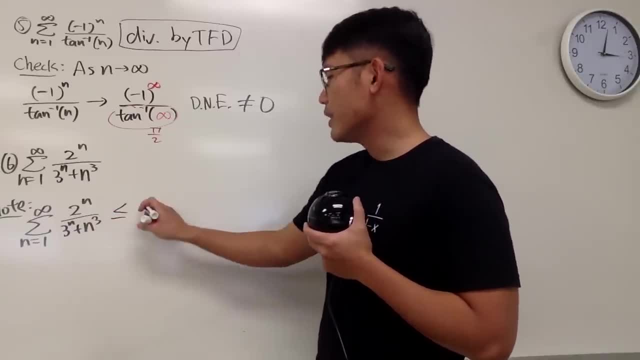 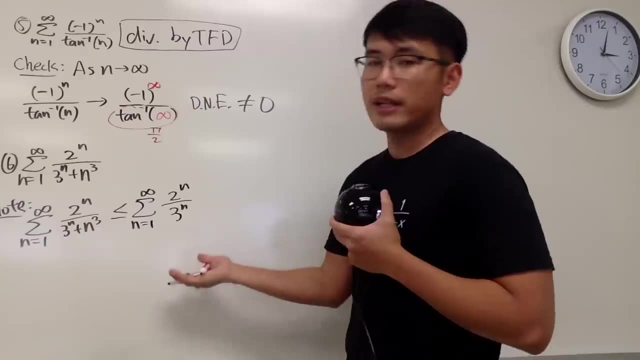 it goes. Anyway, get rid of that and we can say: this is the sum as n goes from one to infinity, which is two to the nth power over three to the nth power. like that. This guy is bigger than that. This guy is less than that. 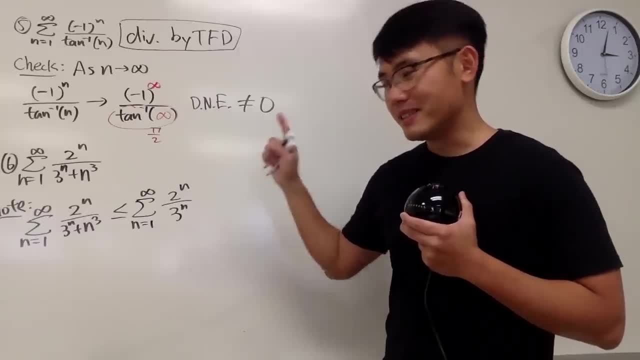 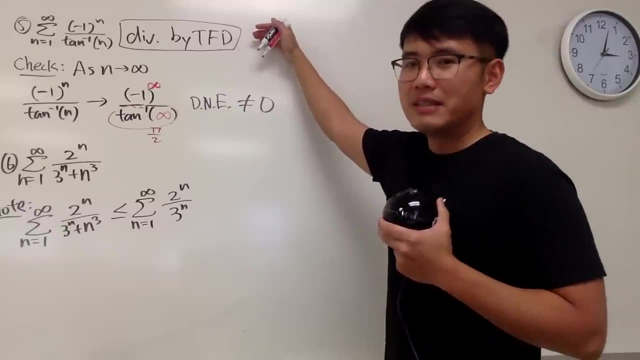 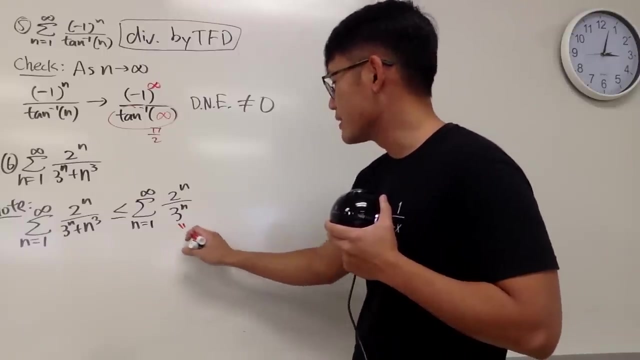 This is not hard because it's easy. Please do not say this right here: diverges because it does not converge. Please do not say that. Anyway, here we go, This right here. the truth is, of course, we can write this down as: 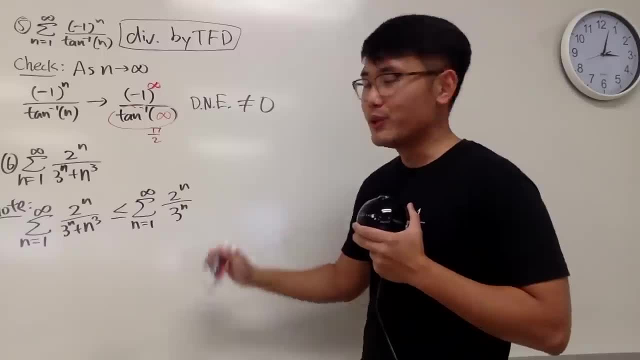 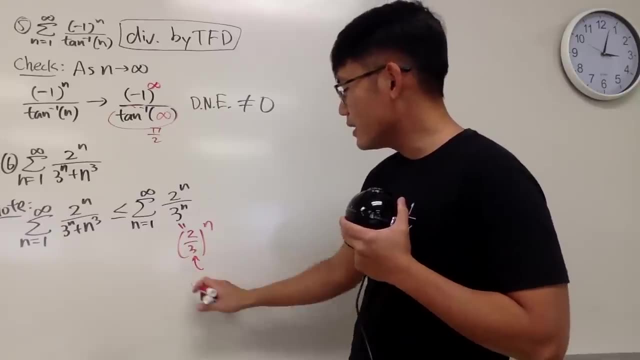 Please don't. Anyway, here we go, This right here. the truth is, of course, we can write this down as 2 over 3 to the nth power, and the idea is: notice r is equal to 2. third, This is the geometric series, and. 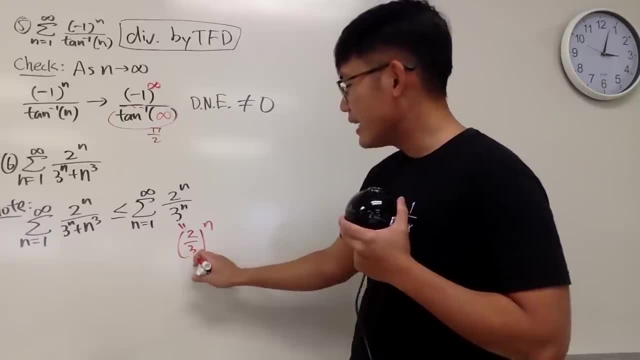 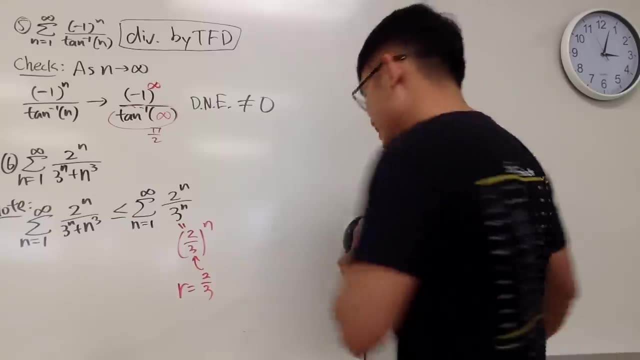 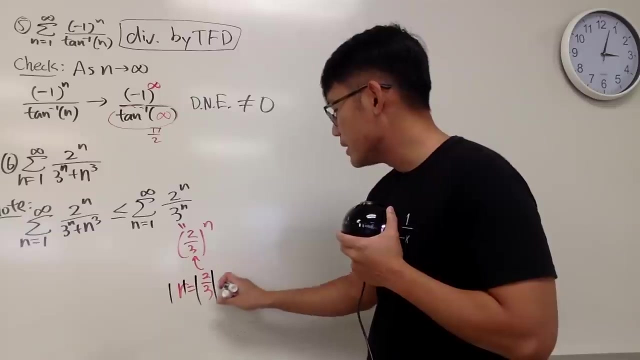 two over three to the nth power, and the idea is: notice, r is equal to two-third. This is the geometric series and, yes, this is our best friend right here, But anyway, you have to remember the absolute value of r has to be less than. 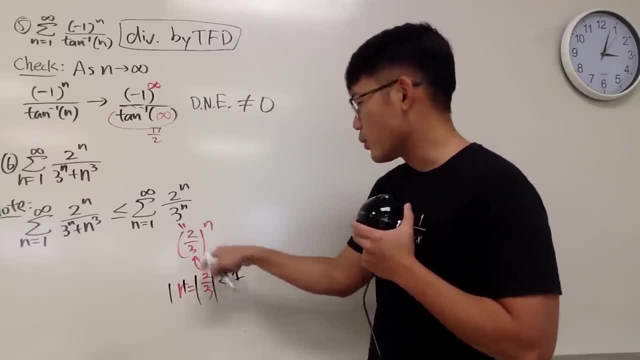 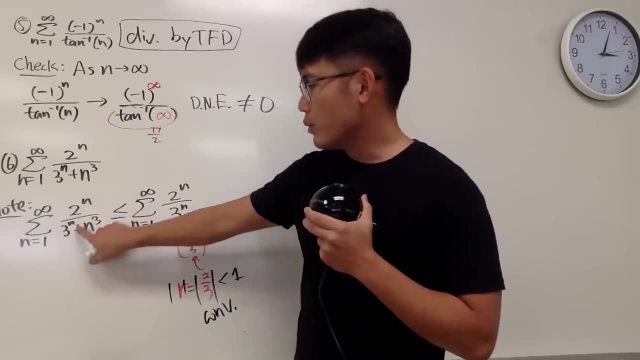 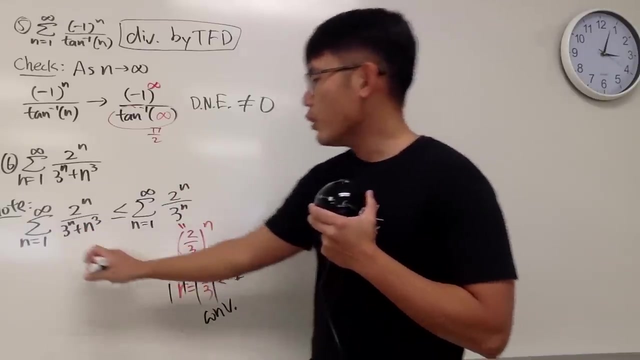 one in order for this to converge. and it is less than one. so we know this guy converges. And we do have this inequality, because when you have a smaller denominator, this is bigger. right, You can just remove that. So we can. 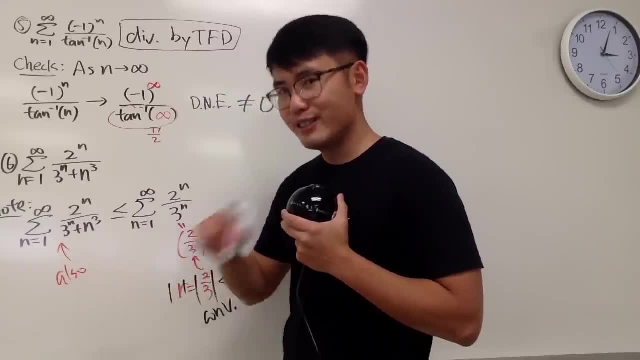 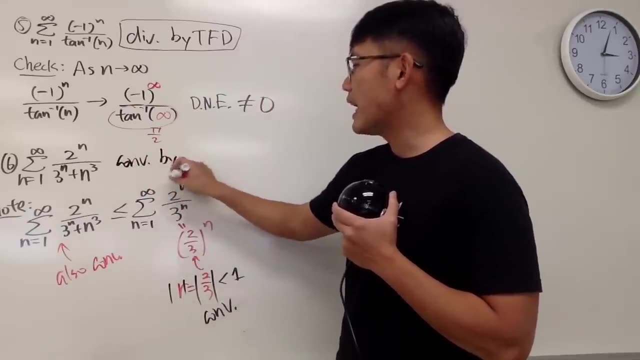 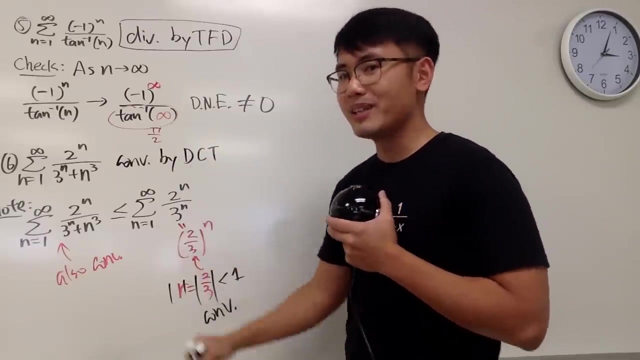 conclude that this right here also what Converges, Nice, So I'll come here and say this right here actually converges by test, No, sorry, by d, which is direct comparison test, because again inequality Converges. 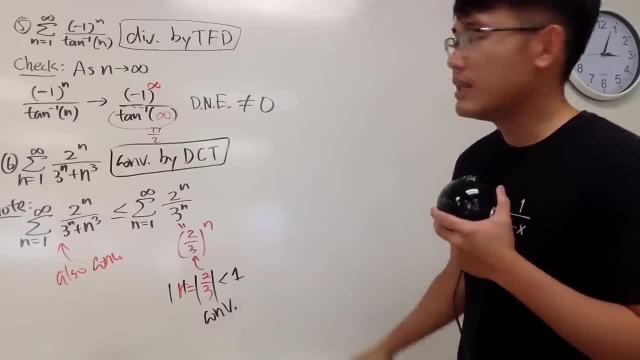 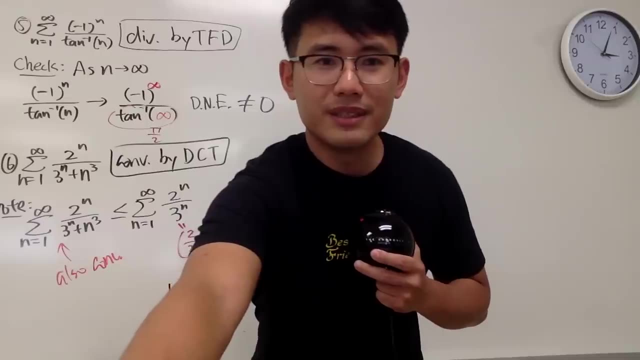 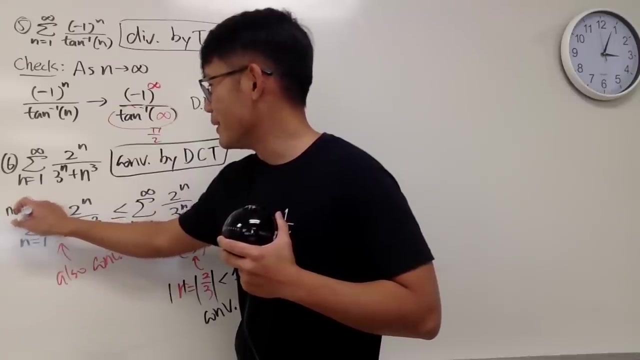 by direct comparison test, And that's it Okay. Note, note, note, Okay, Like that a little bit. Oh, yeah anyway. Hmm, I am not going to pause the video and then do it, So note. 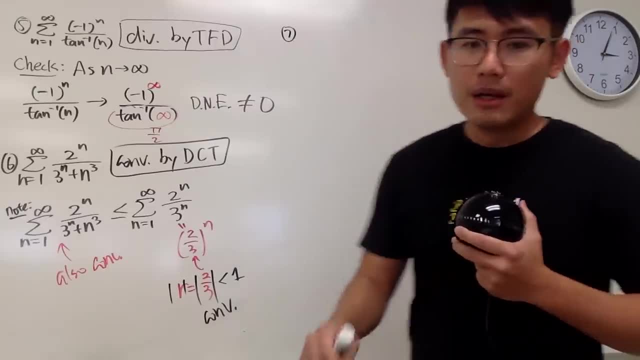 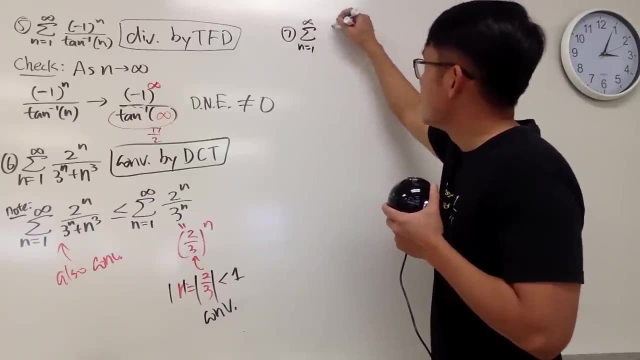 Okay, now number seven, Slightly different, So pay close attention to this. This time we have n on the top, so we have the sum as n goes from 1 to infinity. Here we have 3 to the n over. 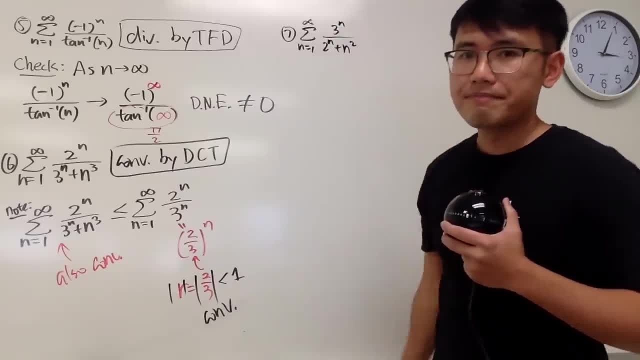 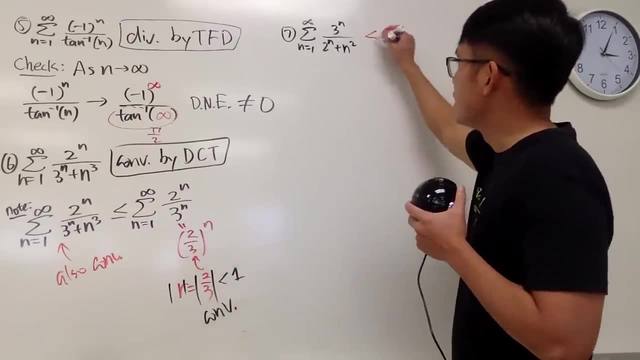 2 to the n plus n squared like that. Well, if you want to do this, let me show you This is actually not good. If you put on less than or equal to ignore the n squared, which you get the sum as n. 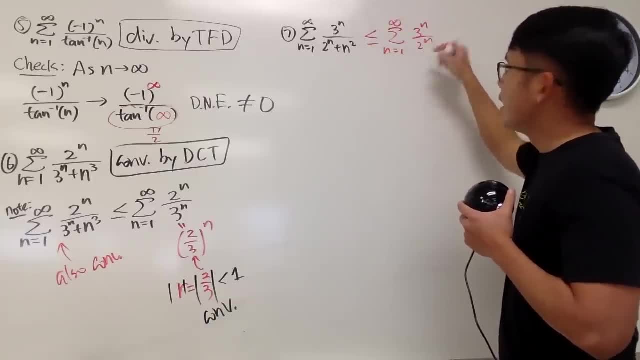 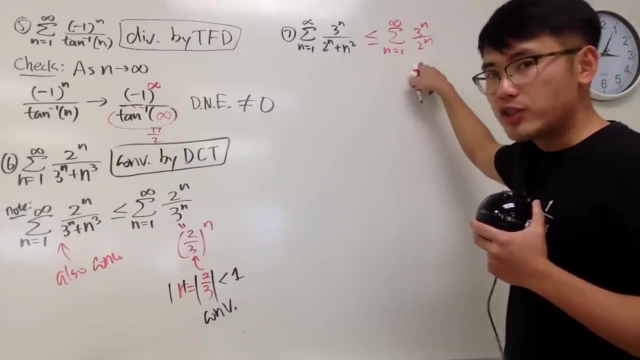 goes from 1 to infinity, 3 to the n over 2 to the n. Okay, This inequality is true, but this right here, the common ratio is 3 over 2.. This is r, is 3 over 2, which is: 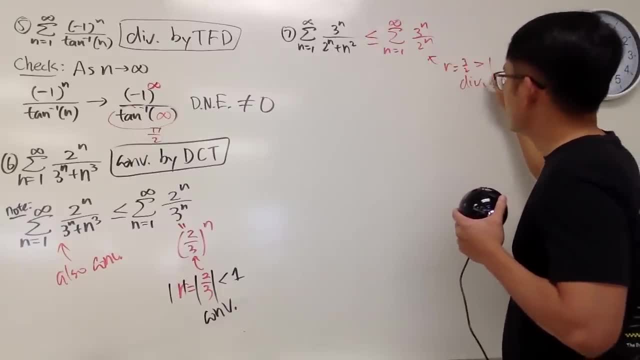 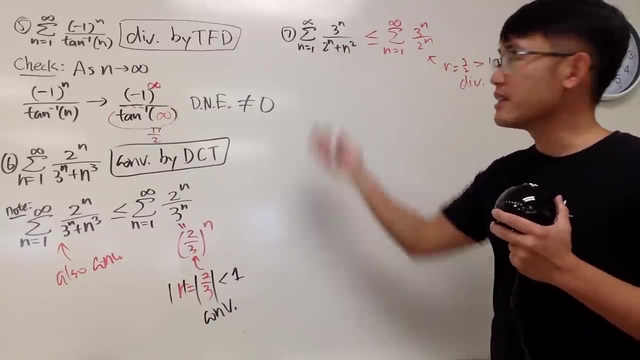 greater than 1, meaning that this right here diverges, And when we have a series that's less than a divergent, we cannot say anything. Again, we are saying: a person is younger than an old person. In that case, we cannot. 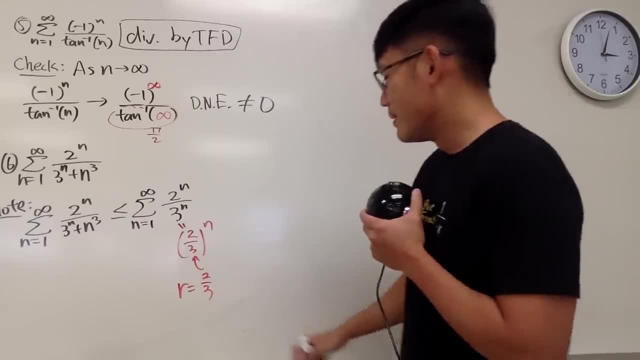 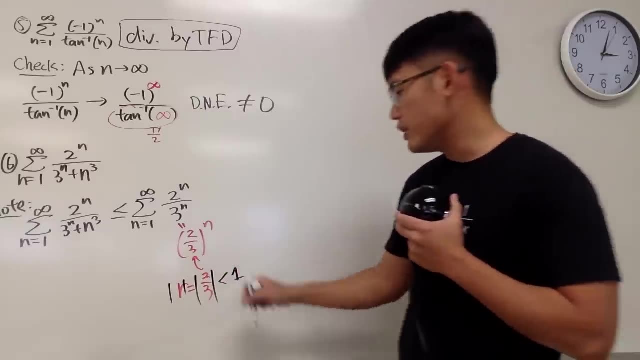 yes, this is our best friend right here, But anyway, you have to remember, the absolute value of r has to be less than 1, in order for this to converge. and it is less than 1.. So we know this guy. 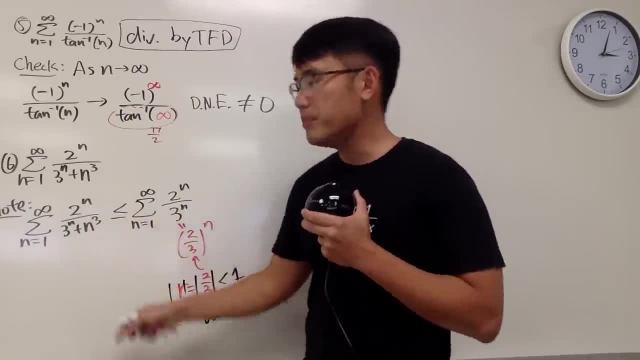 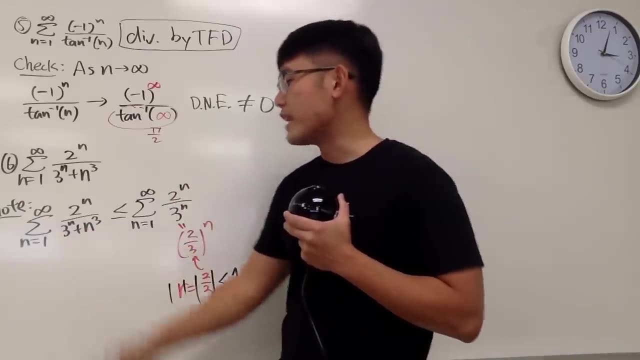 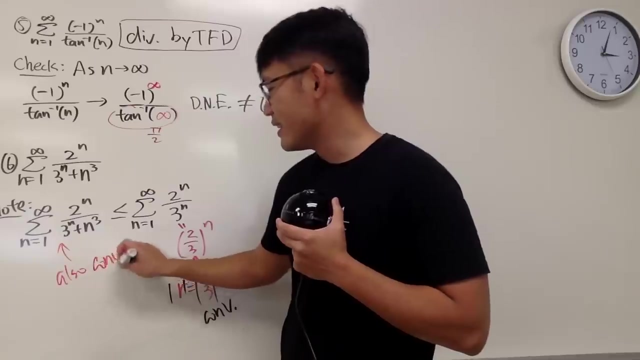 converges And we do have this inequality, because when you have a smaller denominator, this is bigger, right, You can just remove that, So we can conclude that this right here also what Converges, Nice. So I'll come here and say this: right. 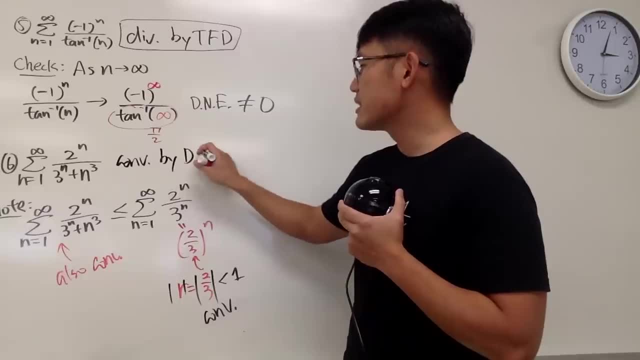 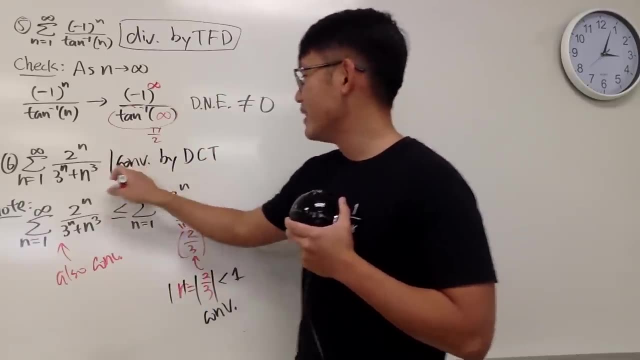 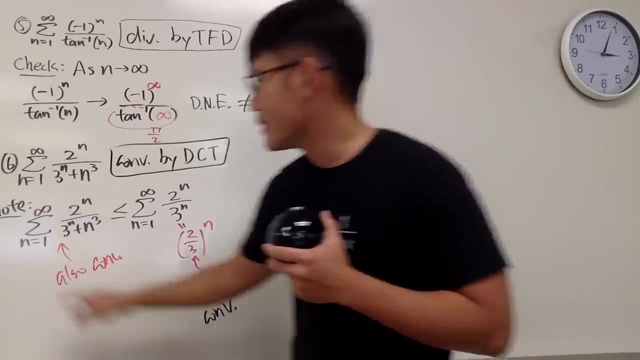 here actually converges by test, No, sorry, by d, which is direct comparison test, Because again, inequality converges by direct comparison test, And that's it Okay. Note, note, note, Okay, Like that a little bit. 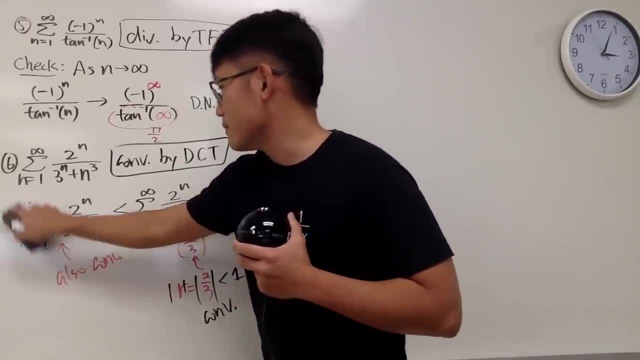 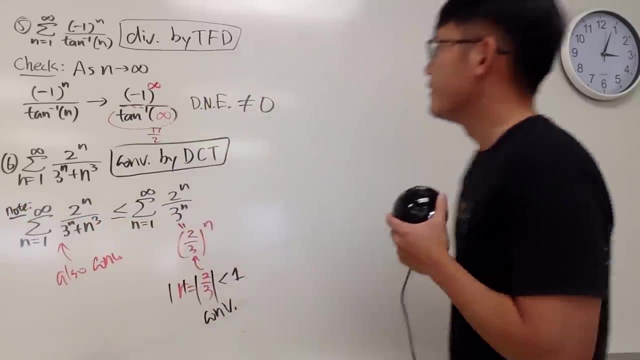 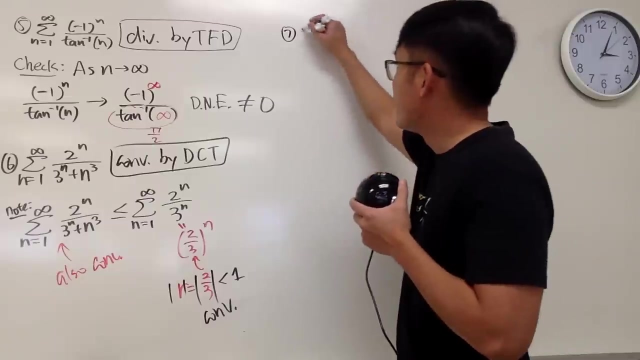 Oh, yeah, anyway. Hmm, I am not going to pause the video and then do it, So note. Okay, now number 7.. Slightly different, So pay close attention to this. This time we have 3 to the n on the top, So we have the. 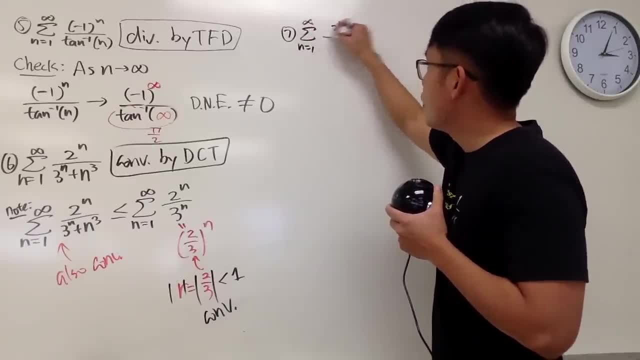 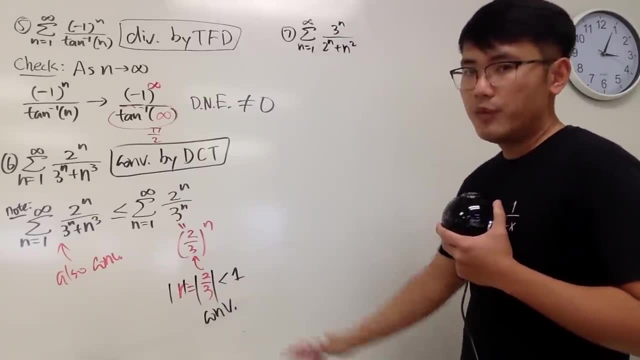 sum as n goes from 1 to infinity. Here we have 3 to the n over, 2 to the n plus n, squared Like that. Well, if you want to do this, let me show you. This is actually not good If you put down less than. 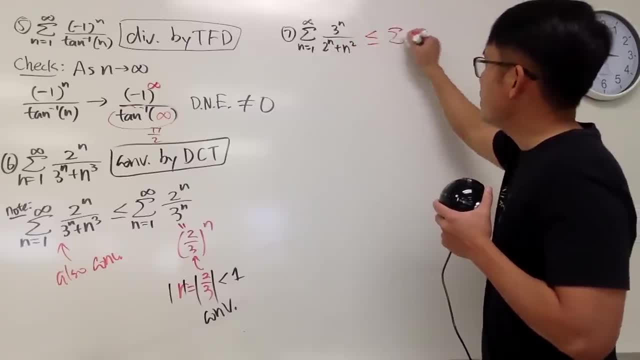 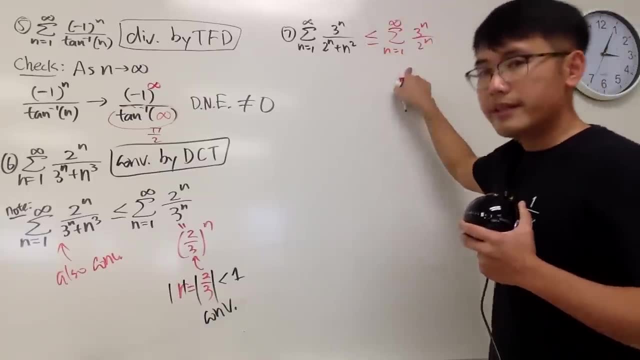 or equal, to ignore the n squared which you get, the sum as n goes from 1 to infinity, 3 to the n over 2 to the n. Okay, This inequality is true, but this right here, the common ratio is 3 over 2.. 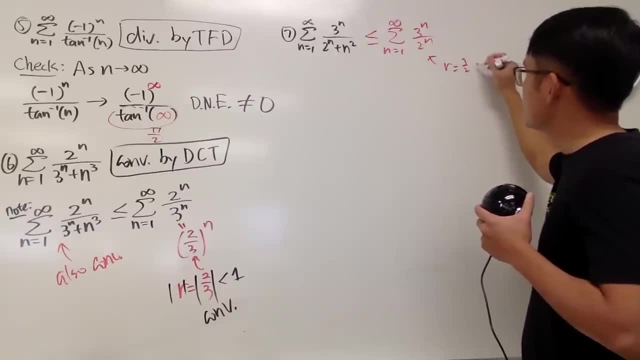 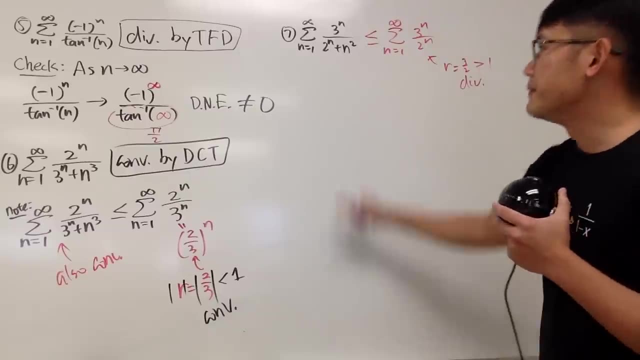 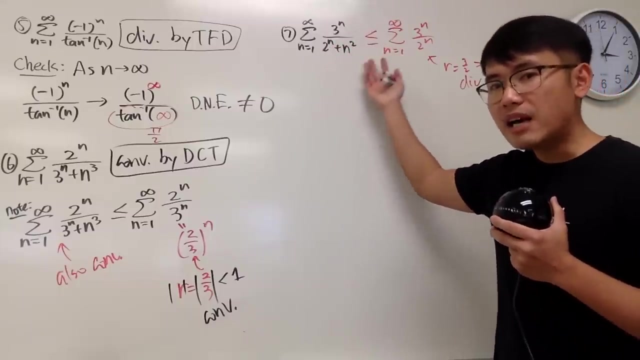 This is r, is 3 over 2,, which is greater than 1, meaning that this right here diverges, And when we have a series that's less than a divergent, we cannot say anything. Again, we are saying: a person is younger than. 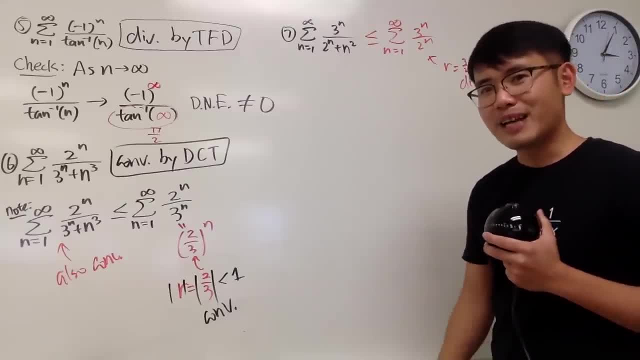 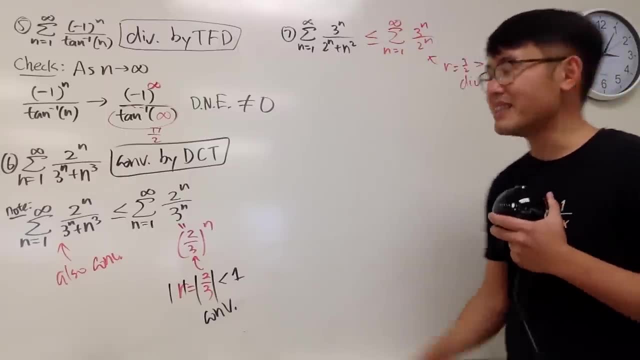 an old person. In that case we cannot draw any conclusion about that. It's like if you guys are saying you guys are younger than me, Well, I'm young, so you guys can say you are young. but if you have a 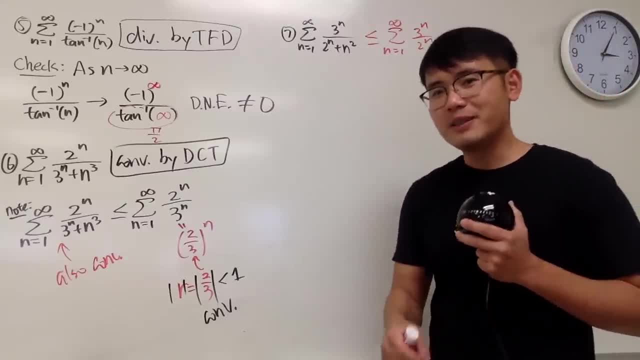 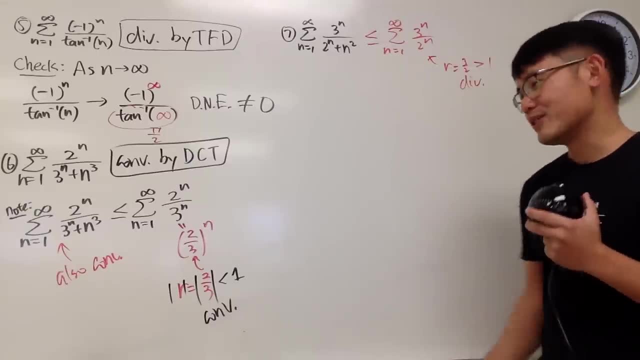 draw any conclusion about that. It's like if you guys are saying you guys are younger than me, Well, I'm young, so you guys can say you are young, but if you have a divergent, then we cannot say anything. 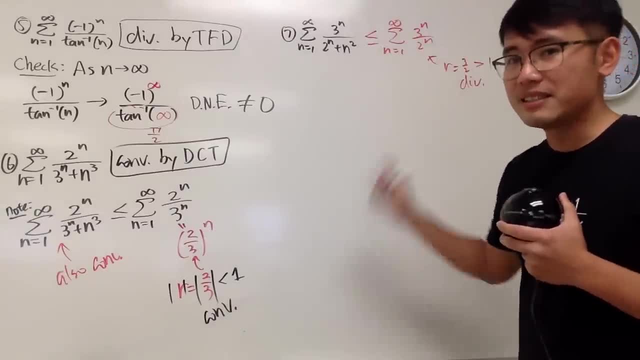 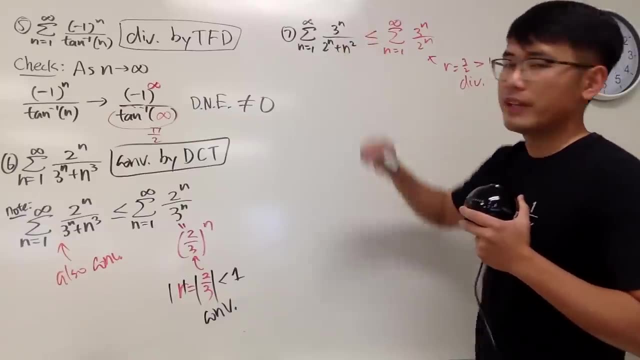 So, unfortunately, the direct comparison test- it does not work out nicely like this. alright, Hmm, Again, we are going to think about the dominating part, which is just this, over that. So we are still going to be using this, And now we will be. 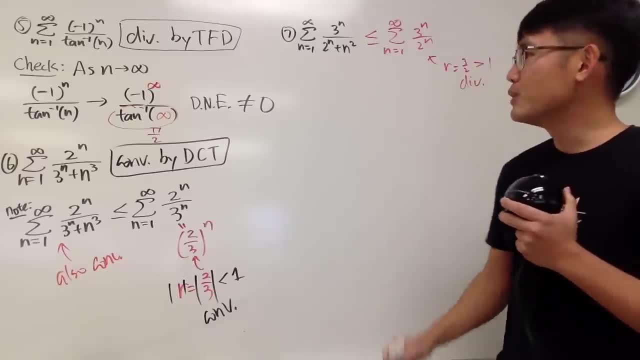 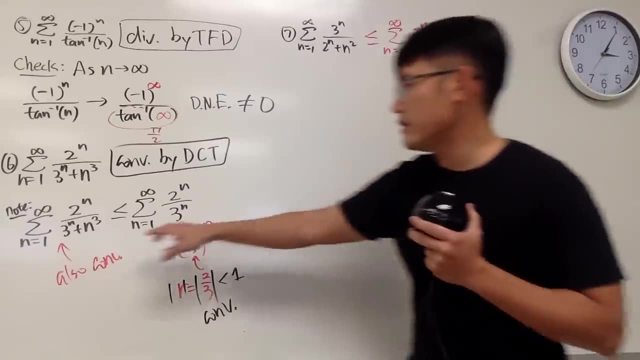 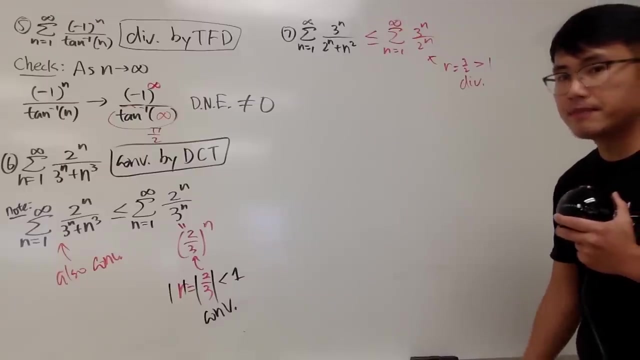 doing the limit version of the comparison test, which is still just as powerful Sometimes, if the inequality does not work out this well, and if the inequality does not work out this well, then in that case we'll just try the limit comparison test. 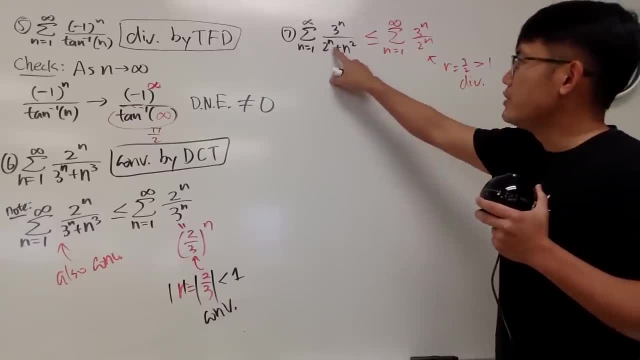 Okay, here's the deal. In fact, if you change this to minus and then this will be greater than or equal to, that will work out nicely. But again, if you just want to look at this question, no right. 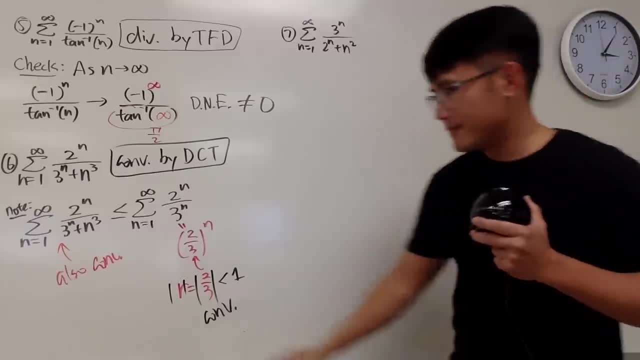 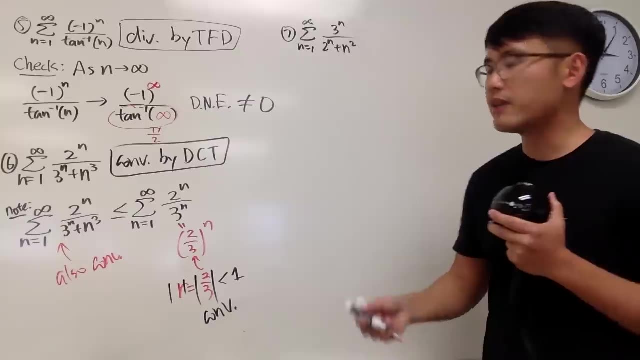 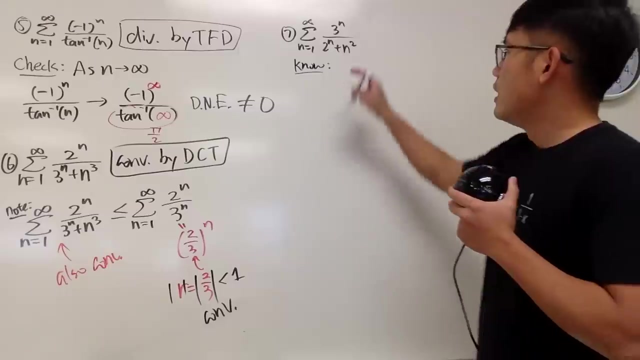 So let me erase this. Hmm, Let me see. This is the three steps I would like to do to make things clear for my students. Sometimes I think, if I want to make things more clear, then I'll just do this. 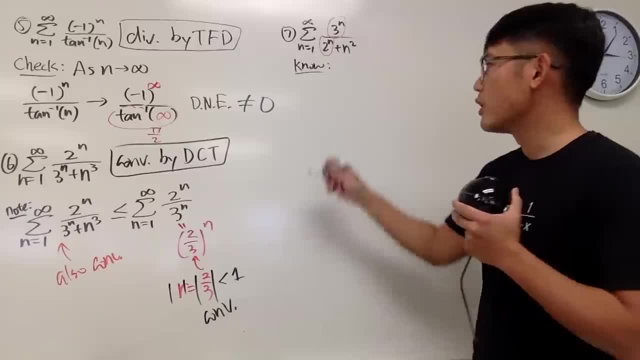 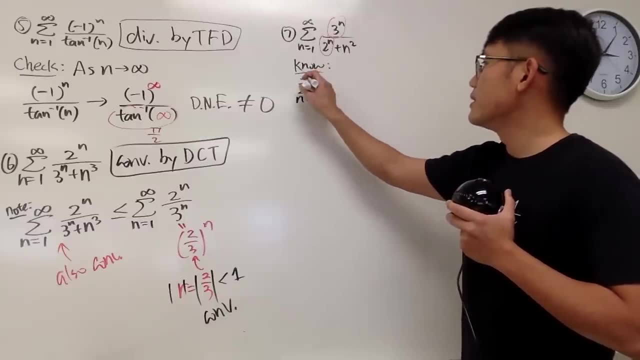 First of all, I know to pick the dominating part. So we know the sum as n goes from 1 to infinity. ah, infinity, right here. infinity stone. 3 to the n over 2 to the n. We know this right here. 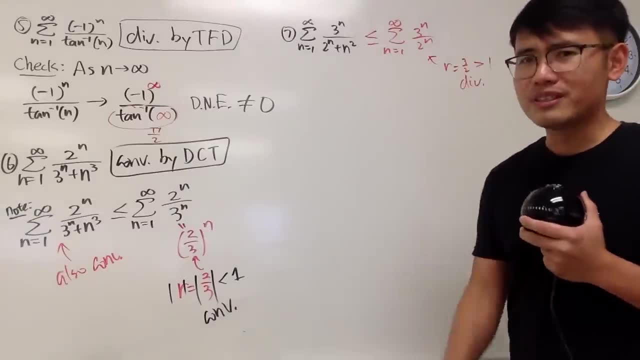 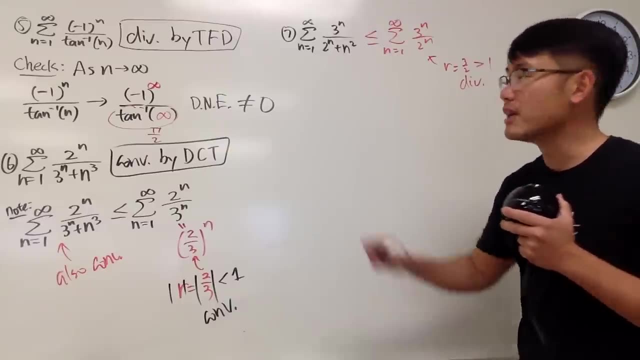 divergent, then we cannot say anything. So, unfortunately, the direct comparison test: it does not work out nicely like this. Alright, Hmm, Again, we are going to think about the dominating part, which is just this over that. So we are still going to be using 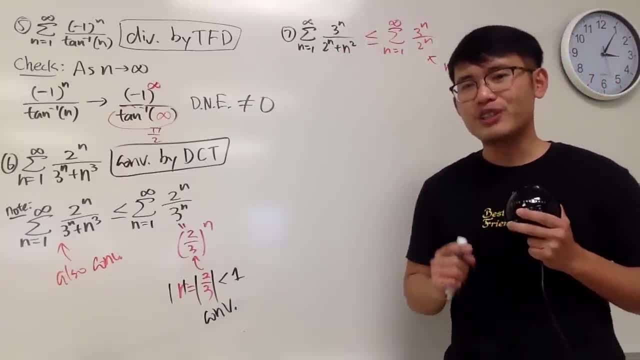 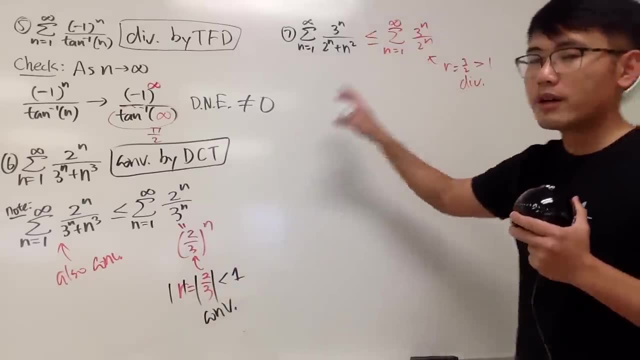 this, And now we will be doing the limit version of the comparison test, which is still just as powerful Sometimes, if the inequality does not work out this well, if the inequality does not work out this well, then in that case, 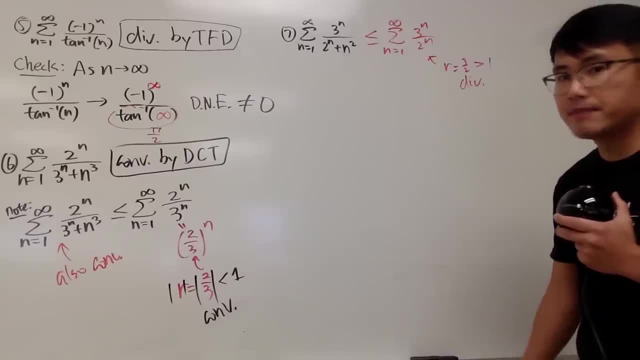 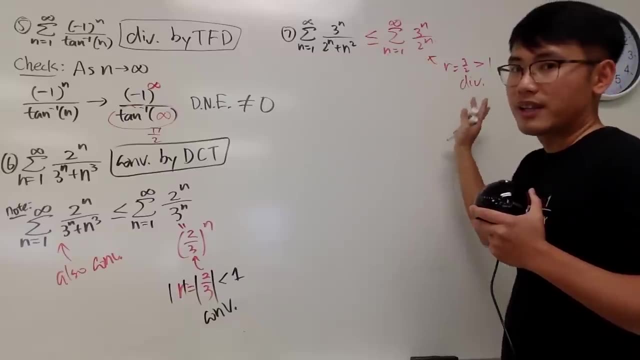 we'll just try the limit comparison test. Okay, here's the deal. In fact, if you change this to minus and then this will be greater than or equal to, that will work out nicely. But again, if you just want to look at this question, no right. 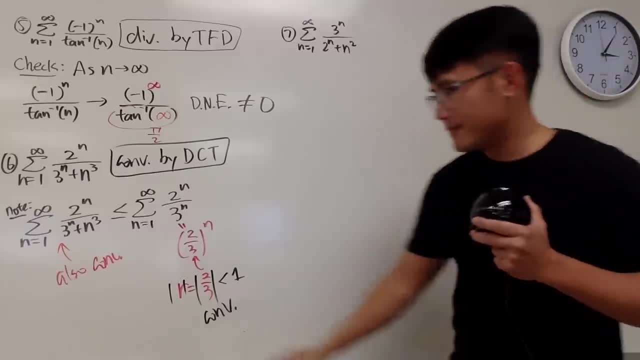 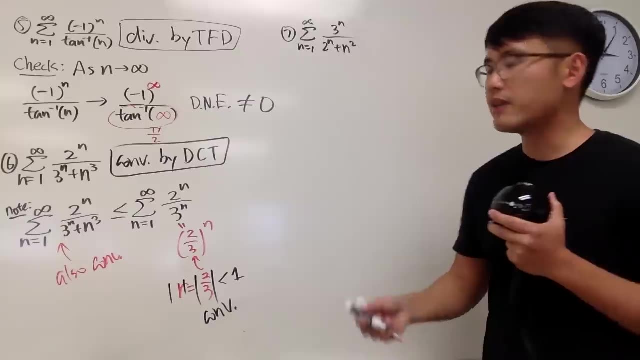 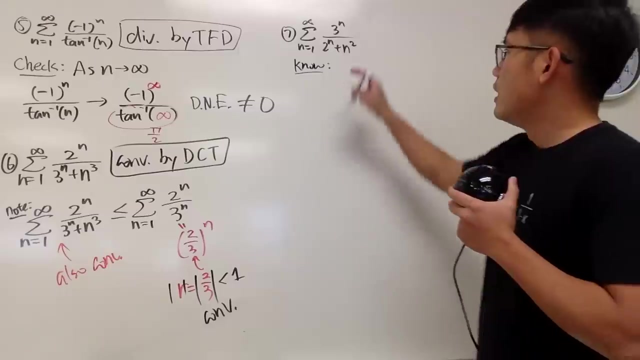 So let me erase this. Hmm, Let me see. This is the three steps that I would like to do to make things clear for my students. Sometimes I think, if I want to make things more clear, then I'll just do this First. 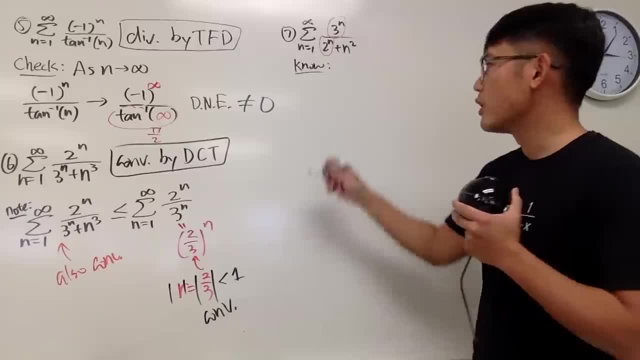 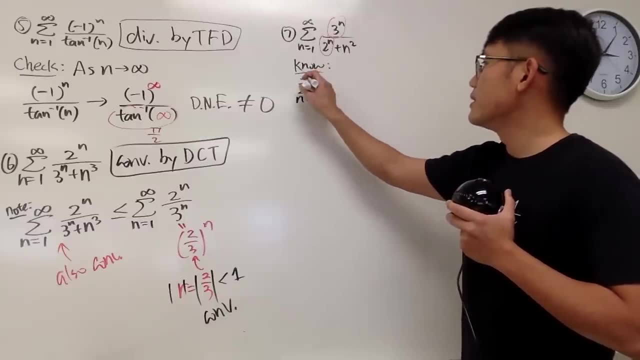 of all I know, to pick the dominating part. So we know the sum as n goes from 1 to infinity- Uh, infinity, right here. Infinity stone. 3 to the n. over 2 to the n. We know this right here. 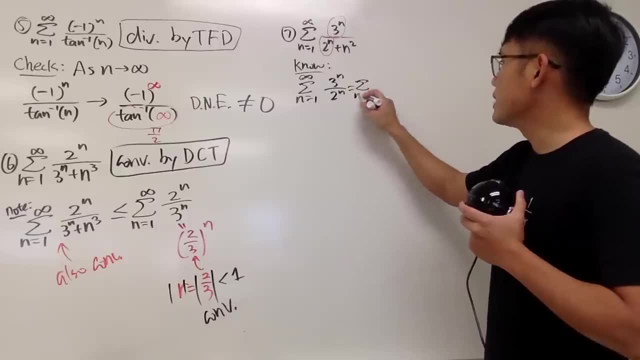 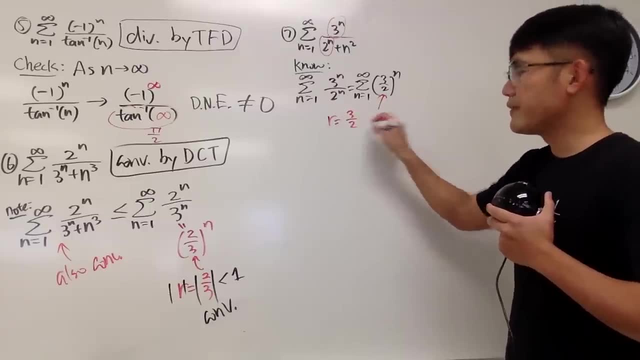 which is just put this down: the sum as n goes from 1 to infinity, 3 over 2 to the nth power, As we all know this right here, r is 3 half, But again, if you take the absolute value of r, this is bigger. 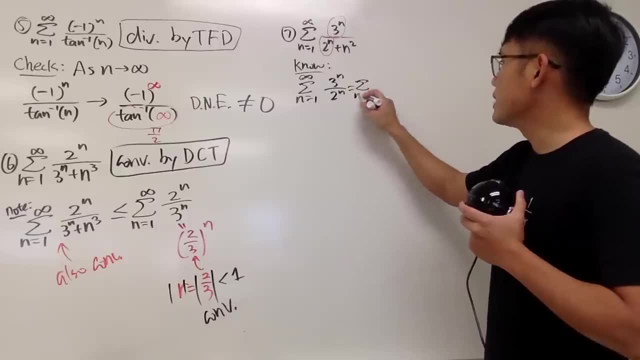 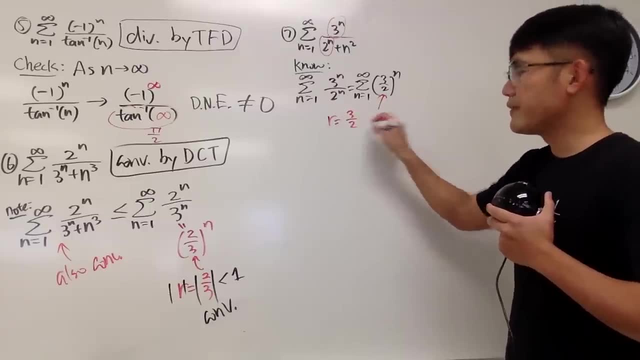 which is just put this down: the sum as n goes from 1 to infinity, 3 over 2 to the nth power, As we all know this right here, r is 3 half, But again, if you take the absolute value of r, this is bigger. 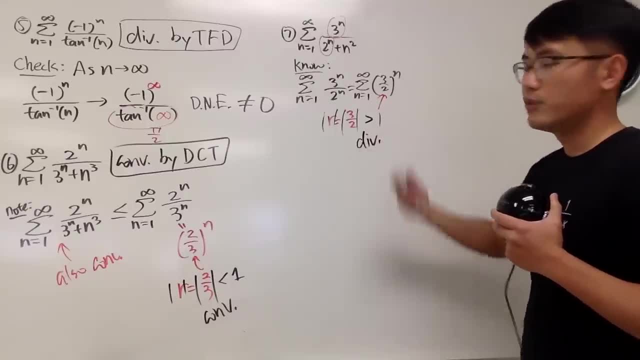 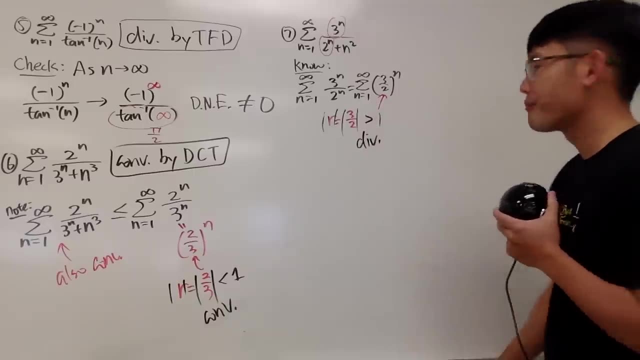 than 1.. So this right here diverges. We're writing down the work to present it to our teachers, and our teachers will be happy and you'll be happy too. Alright, so we write this down. Well, we know this. this right here diverges. 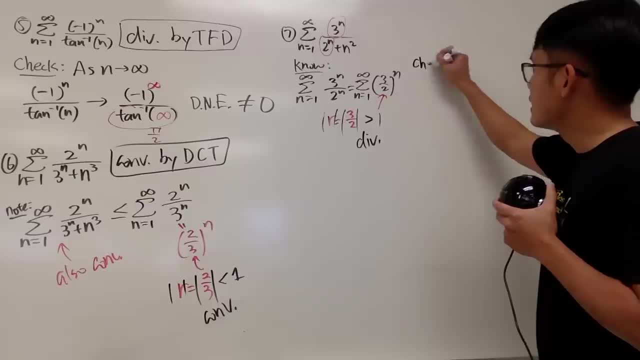 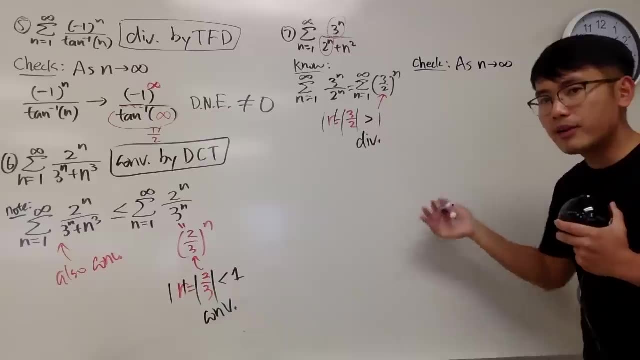 Then what we do next is we are going to check the limit And to do so, we are going to take the limit and we'll just put down as n goes to infinity. I'm not going to put down the l? i n okay. 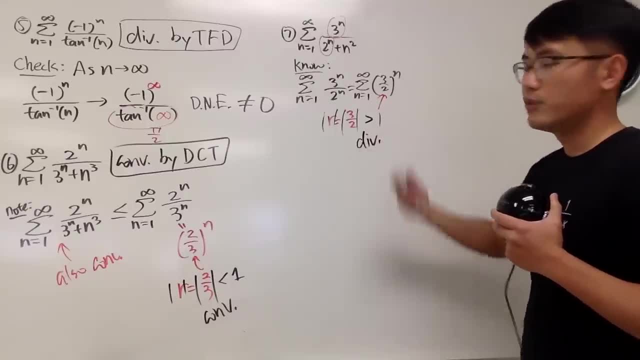 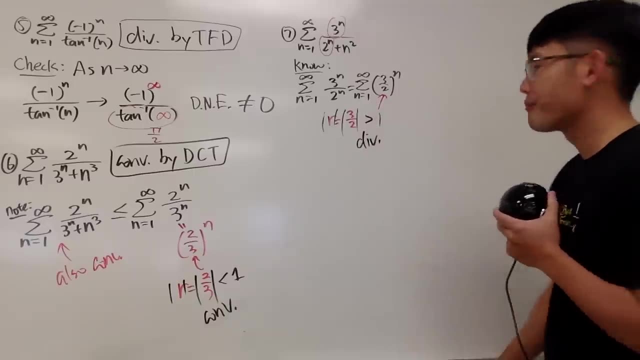 than 1.. So this right here diverges. We're writing down the work to present it to our teachers, and our teachers will be happy and you'll be happy too. Alright, so we write this down. Well, we know this. This right here diverges. 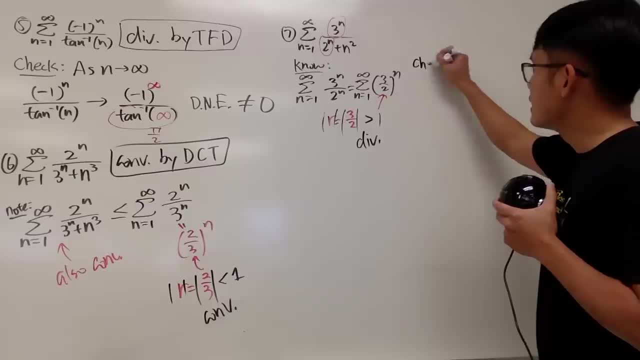 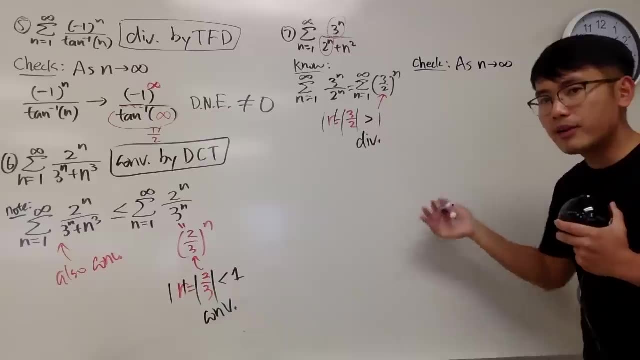 Then what we do next is we are going to check the limit And to do so, we are going to take the limit and we'll just put this down as n goes to infinity. I'm not going to put down the l i n. 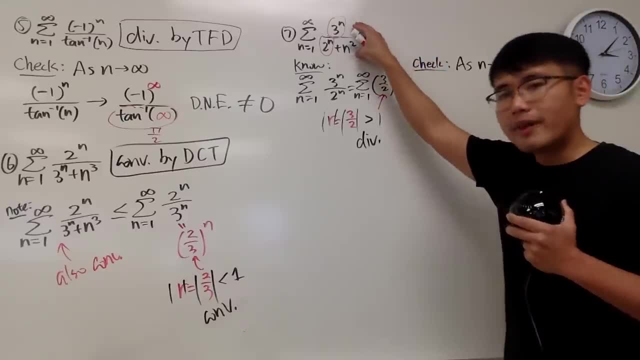 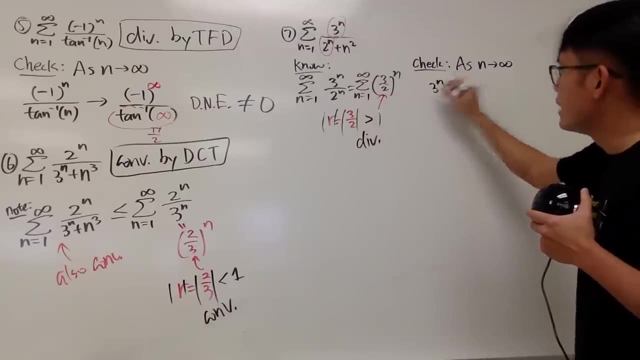 I'll just put this down. I'm going to put down the one that we are doing first on the top And just ignore the sum. we are looking at the a? n part. So let me put down 3 to the n over, 2 to the. 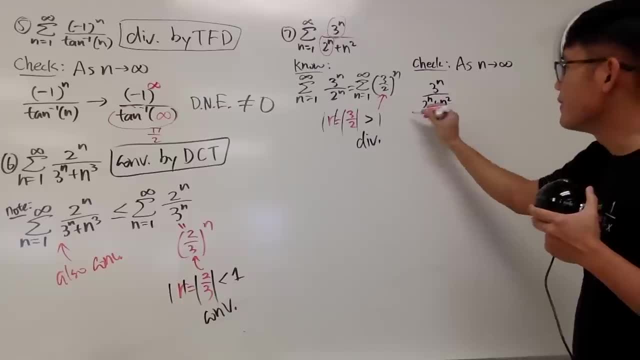 n plus n squared, And then we are going to divide this by the one that we know much better, which is this, And I'll put down this version because it's easier for us to flip earlier. I mean later, It will be easier for us to flip later. 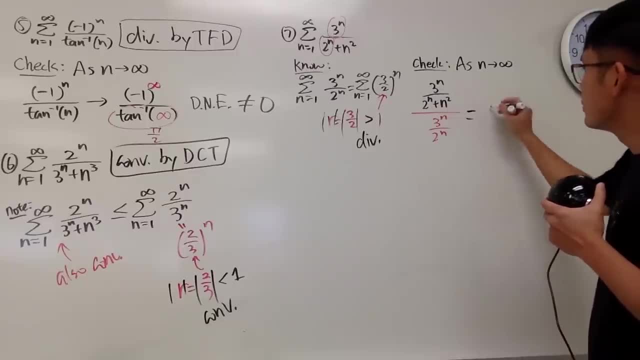 Now let's do algebra. This right here is equal to 3 to the n over 2 to the n plus n squared. And right here we are just doing algebra. so this is the equal sign. Flip this, we get 2 to the n on the top. 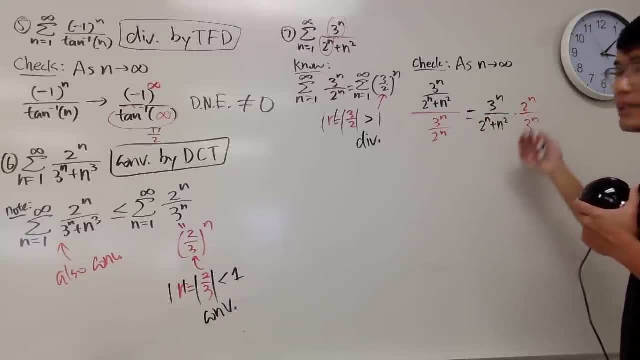 over 3 to the n on the bottom, Isn't it? That's very nice, huh. And now check this out. This and that, cancel out nicely, Huh, Very good. And now we are looking at this as 2 to the n over 2. 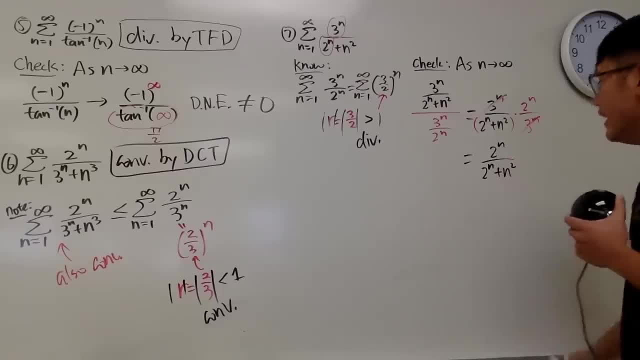 to the n plus n squared Like this, And it depends on your teacher seriously to see how much work you have to show when you are doing limits. In this situation, again, we are comparing infinities and we can actually do this. 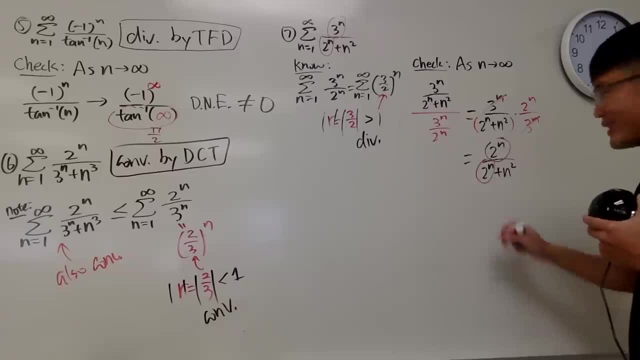 We'll just care about the 2 to the n on the top, 2 to the n on the bottom. so, in other words, this right here approaches 2 to the n over 2 to the n, which is just equal to 1.. 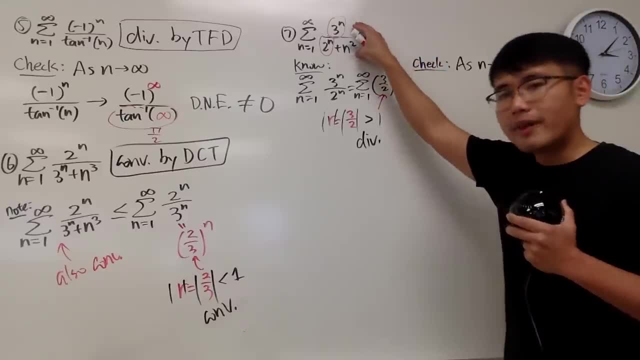 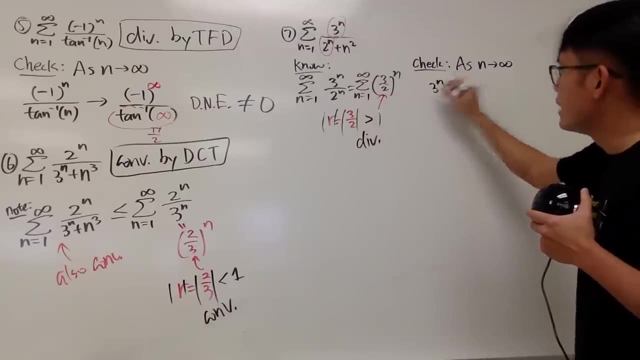 I'll just put this down. I'm going to put down the one that we are doing first on the top And just ignore the sum. we are looking at the a? n part. So let me put down 3 to the n over, 2 to the. 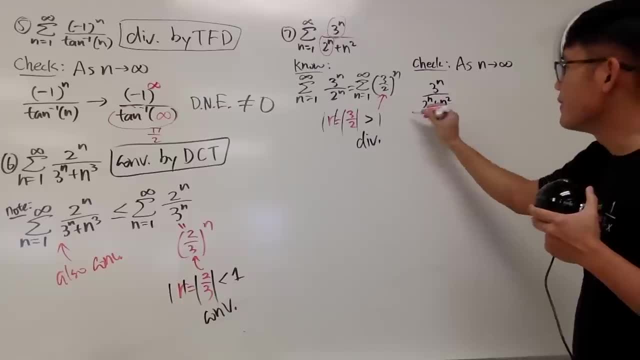 n plus n squared, And then we are going to divide this by the one that we know much better, which is this, And I'll put down this version because it's easier for us to flip earlier- I mean later- It will. 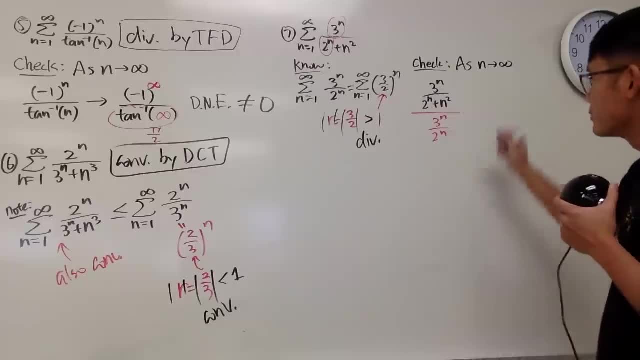 be easier for us to flip later. Now let's do algebra. This right here is equal to 3 to the n over 2 to the n plus n squared. And right here we are just doing algebra. so this is the equal sign. 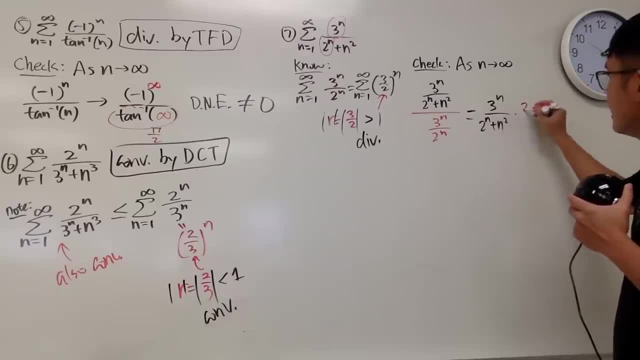 Flip this, we get 2 to the n on the top over 3 to the n on the bottom, Isn't it? That's very nice, huh. And now check this out, This and that. cancel out, nicely, Huh, Very good. 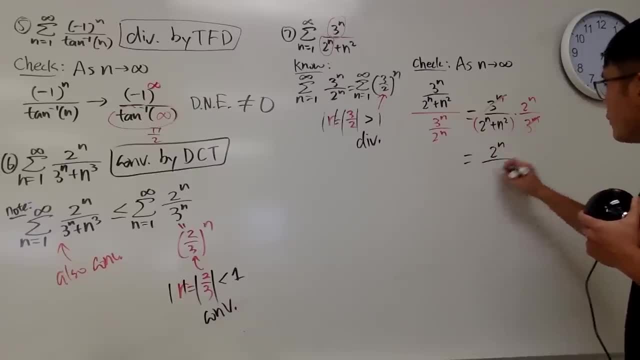 And now we are looking at this as 2 to the n over 2 to the n plus n, squared like this, And it depends on your teacher seriously to see how much work you have to show when you are doing limits In this situation. 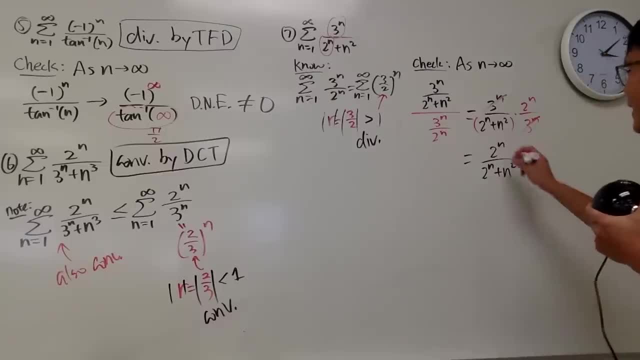 again, we are comparing infinities and we can actually do this. We'll just care about the 2 to the n on the top, 2 to the n on the bottom. So in other words, this right here approaches 2 to the. 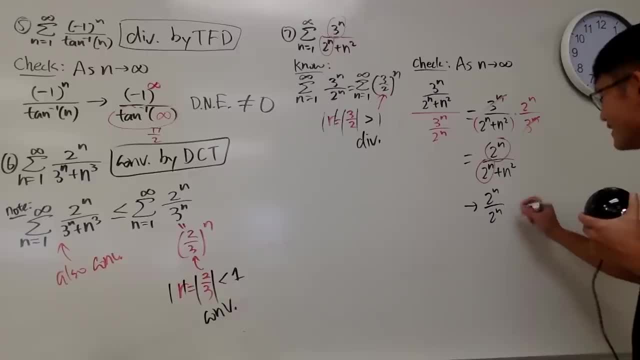 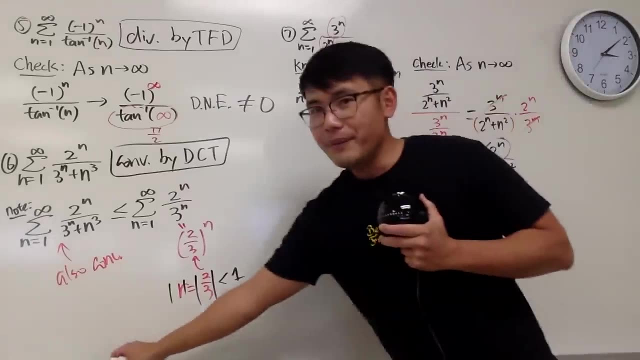 n over 2 to the n, which is just equal to 1.. So the limit is actually equal to 1.. You can do it this way, right? Or you can also divide the top and bottom by 2 to the n's power. 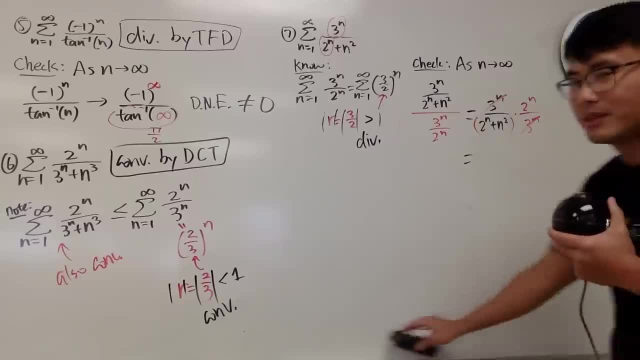 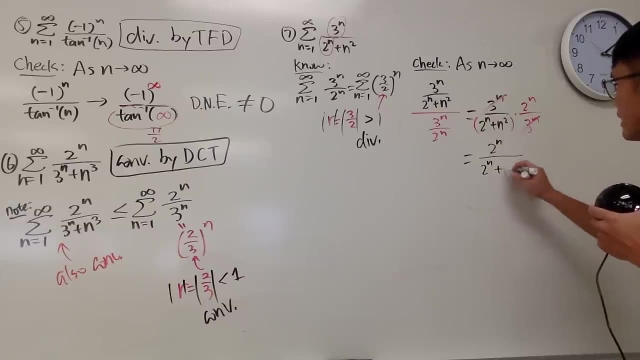 I think I will put that down to be like more legitimate this time right. So 2 to the n over 2 to the n plus n, squared Again. what we do is actually just divide this by 2 to the n. 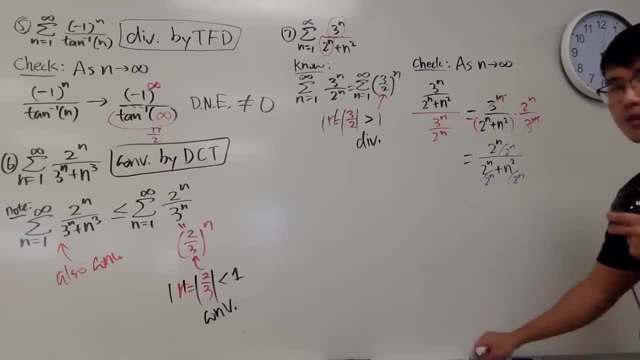 divide everybody by 2 to the n And we are still doing algebra. so this is 1 on the top over 1 right here. plus this is n squared over 2 to the n And by the list you see that this is n to the p's power. 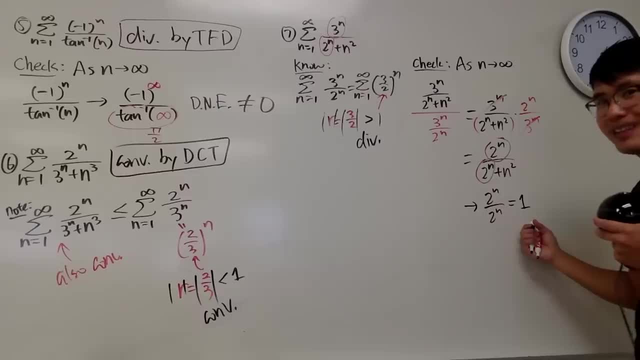 So the limit is actually equal to 1.. You can do it this way, right? Or you can also divide the top and bottom by 2 to the n's power. I think I will put that down to be a little more legitimate. 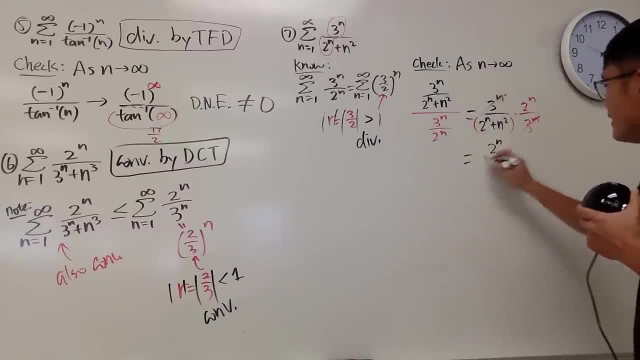 this time right. So 2 to the n over 2 to the n plus n, squared Again. what we do is actually just divide this by 2 to the n, divide everybody by 2 to the n, And we are still doing algebra. so 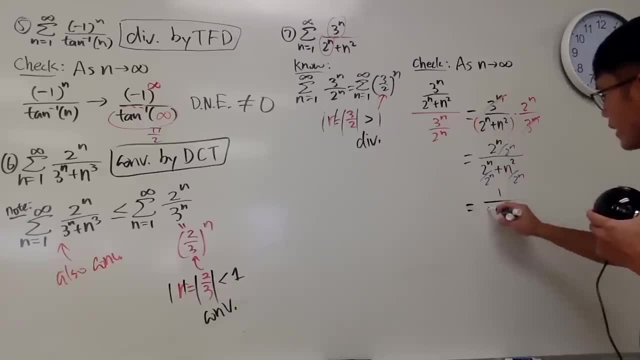 this is 1 on the top over 1 right here. plus this is n squared over 2 to the n And by the list you see that this is n to the p's power over b to the n's power. This is positive power. 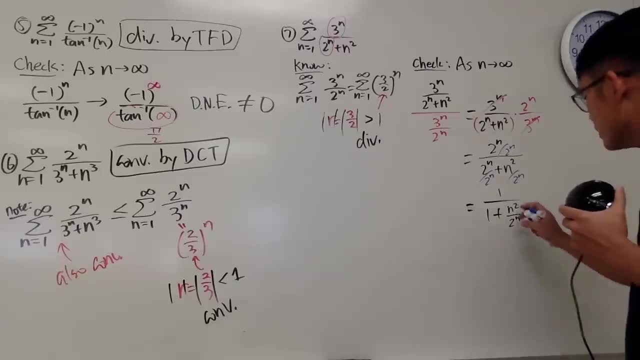 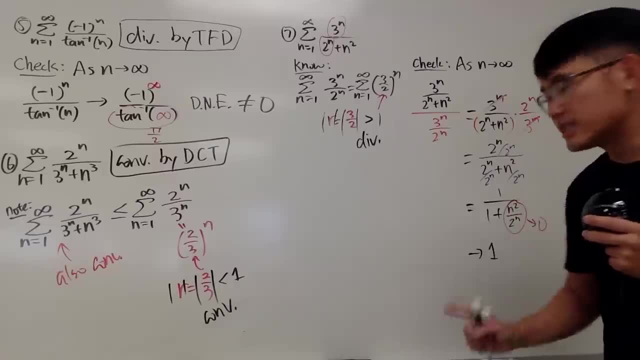 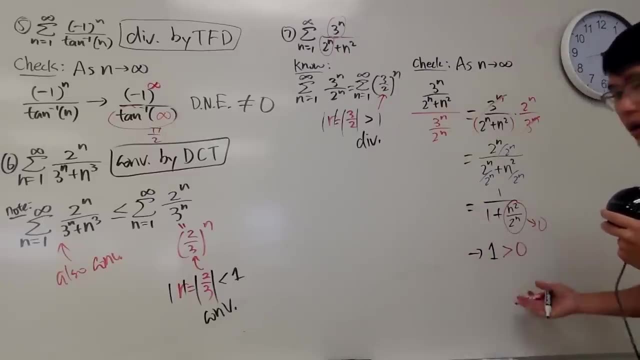 We get 1, and this is the limit comparison test. Does the 1 help us out? Yes, it does. We have to indicate that 1 is bigger than 0. And the idea is that when we have a ratio- because when we divide- 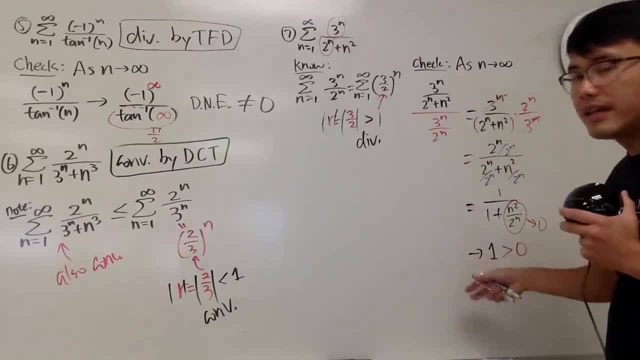 this over that and we get: the limit is equal to 1, in another word, this is about the same size as that, right, Because the ratio is about 1 when n is going to infinity. So this is about the same size as that. 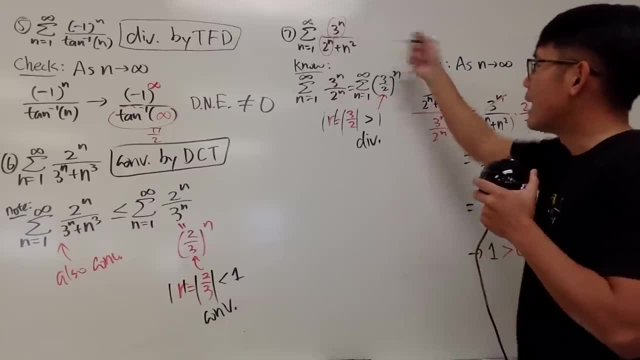 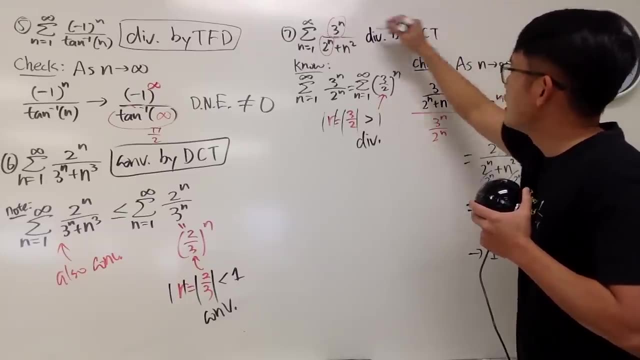 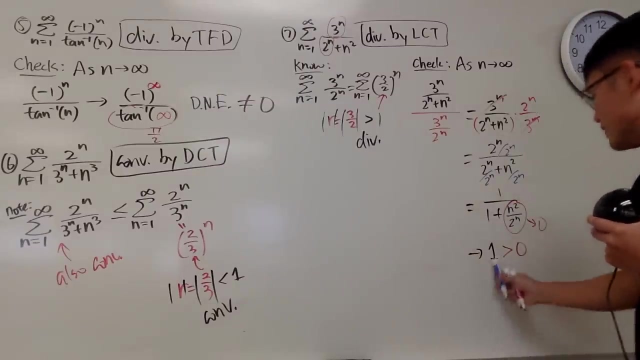 and we know this right here. diverges so we can come back here and say this right here. also diverges by the limit comparison test And with that we are done, Just like that, And we have to be really careful with the number 1,. 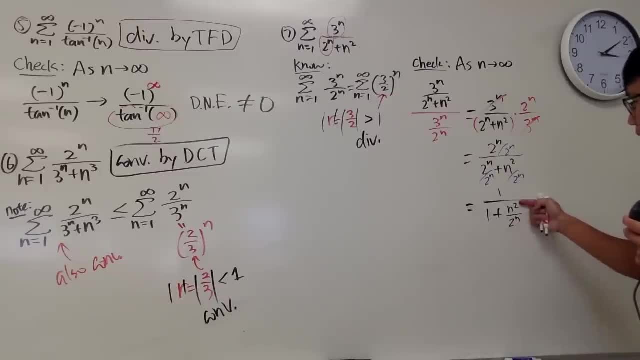 over b to the n's power. This is positive power. this is a base bigger than 1.. From the list: we know this right. here will go to 0.. So in the end, we know this right. here goes to 1, right. 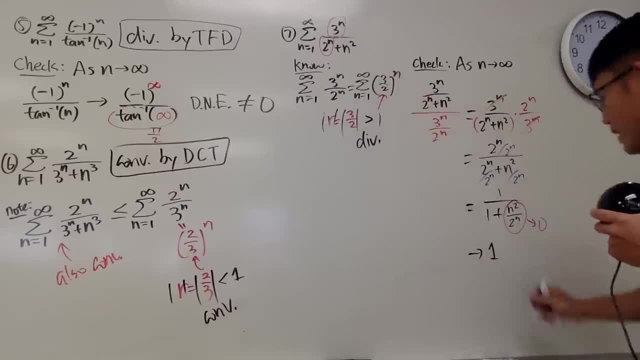 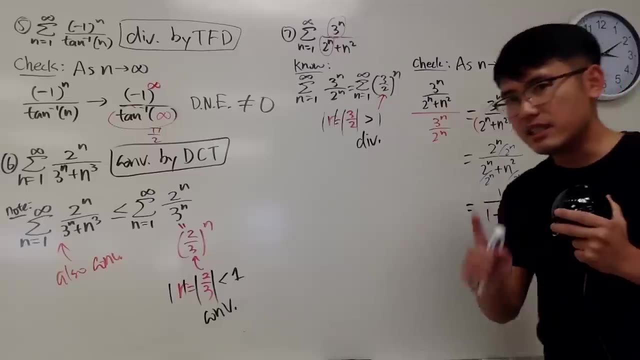 Okay, here's the deal: Blah, blah, blah, blah, blah, blah, blah, We get 1, and this is the limit from Pearson's test. Does the 1 help us out? Yes, it does. We have to indicate that 1 is bigger than. 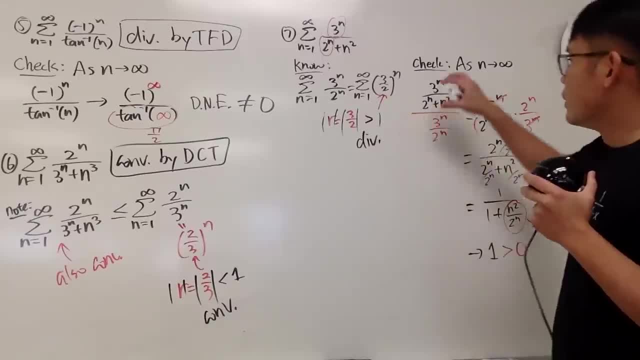 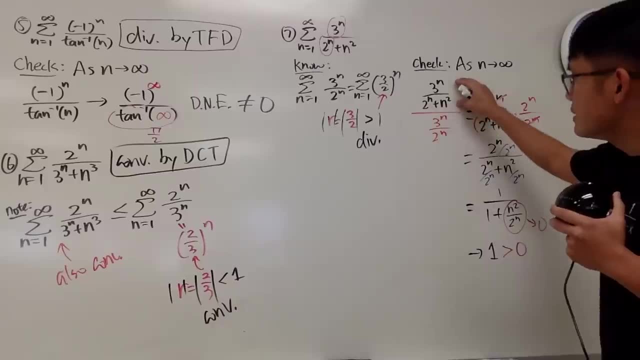 0. And the idea is that when we have a ratio, because when we divide this over that and we get a limit equal to 1, in another word, this is about the same size as that right, Because the ratio is about. 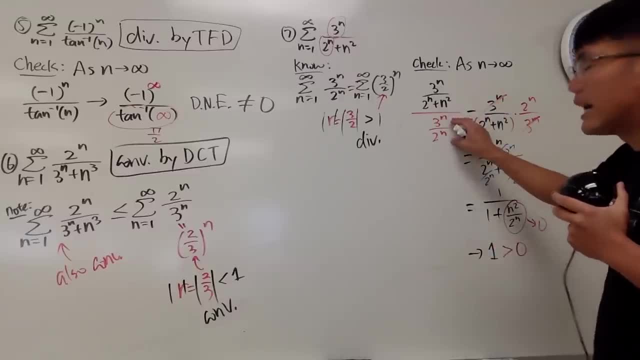 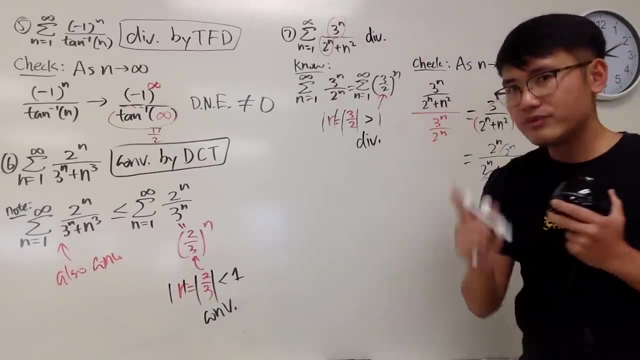 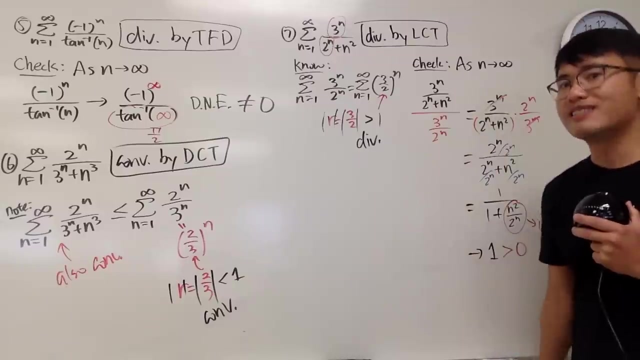 1 when n is going to infinity. So this is about the same size as that and we know this right here. diverges so we can come back here and say this right here. also diverges by the limit from Pearson's test, And with that we are done. 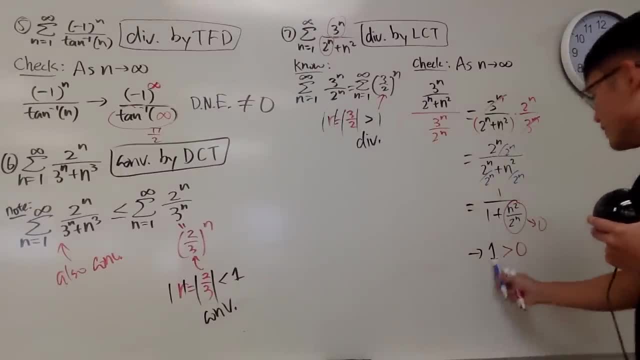 Just like that. And we have to be really careful with the number 1, because sometimes you can use the 1, sometimes you cannot use the 1.. So that's coming up for the ratio test and also the root test. But anyway this, 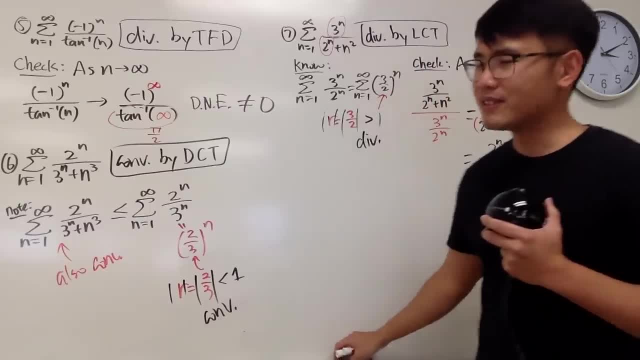 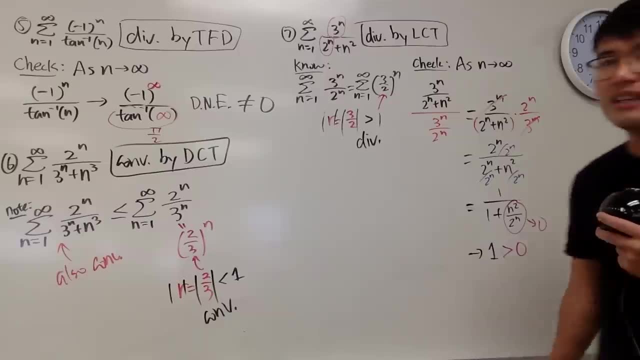 because sometimes you can use the 1,, sometimes you cannot use the 1.. So that's coming up for the ratio test and also the root test. But anyway, this right here, is it Okay? so take a look. 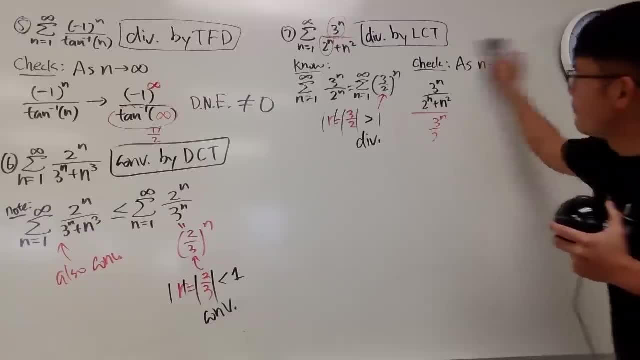 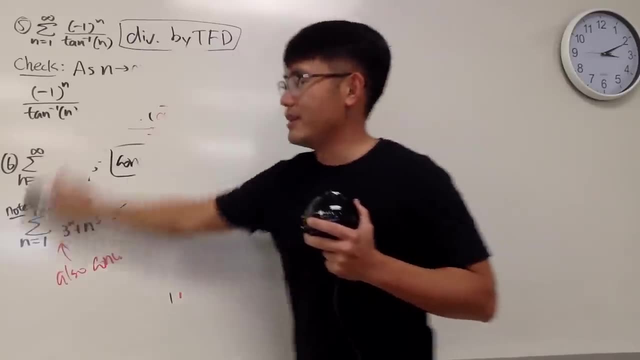 take a look, Okay, so yeah, And you guys can also leave a comment down below. let me know like what school you guys are going to- High school or college- And if you want to give your school a shout out. 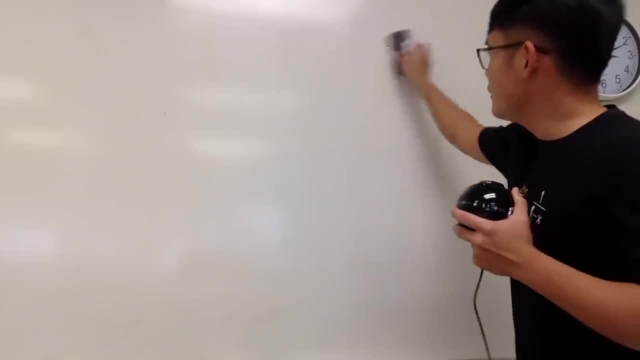 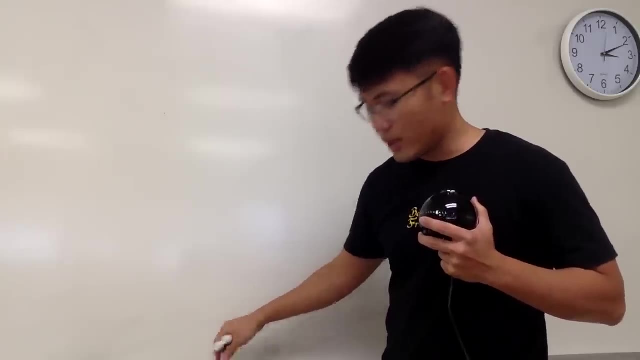 go ahead and do so. Okay, I wonder if there's anybody who goes to like UCLA or like Cal State Northridge? you guys are close by to where I am. that's kind of cool. Maybe I'll meet you guys on the street. 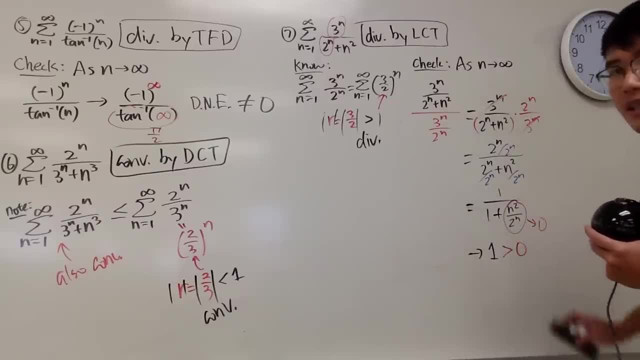 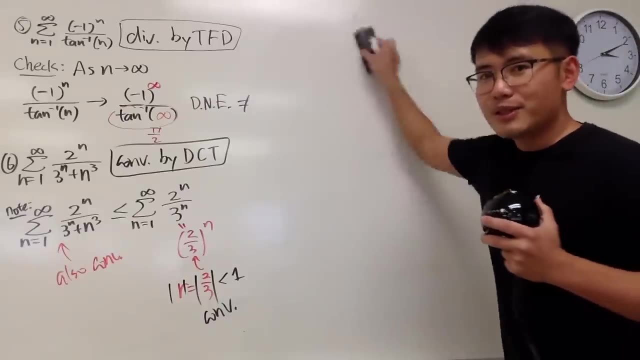 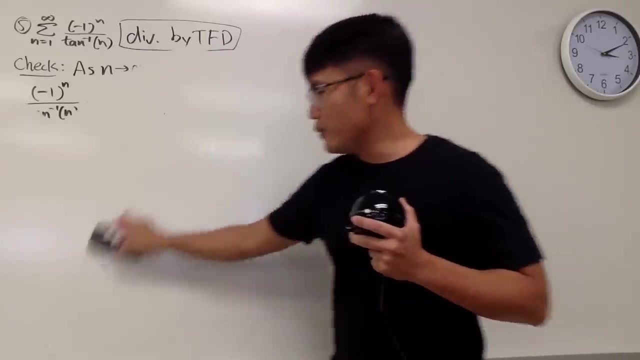 right here is it? Okay? so take a look, take a look. Okay, so yeah, And you guys can also leave a comment down below and let me know like what school you guys are going to- High school or college- And if you want to give your 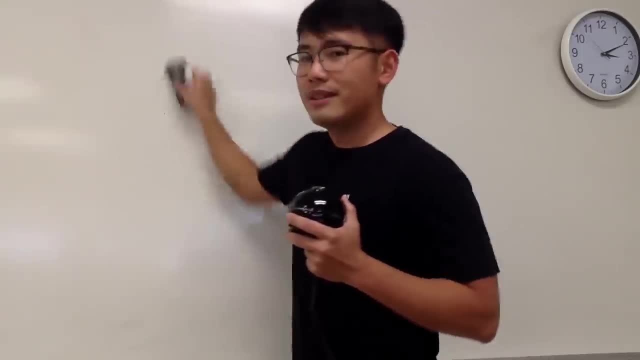 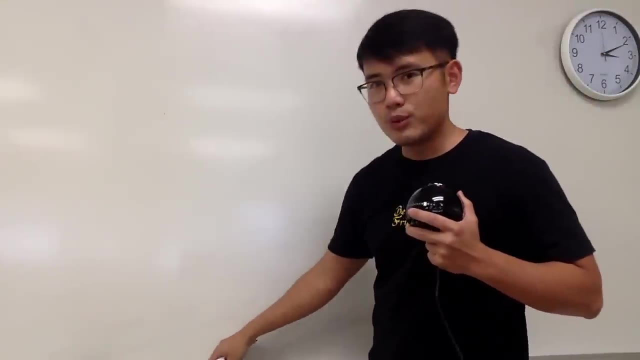 school a shout out. go ahead and do so. Okay, I wonder if there's anybody who goes to like UCLA or like Cal State Northridge? you guys are close by to where I am. that's kind of cool. Maybe I'll meet you guys on the street. 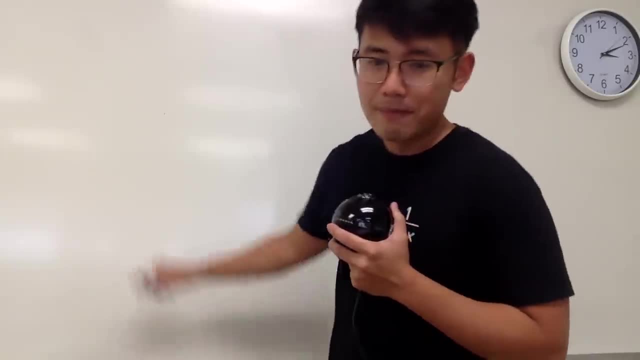 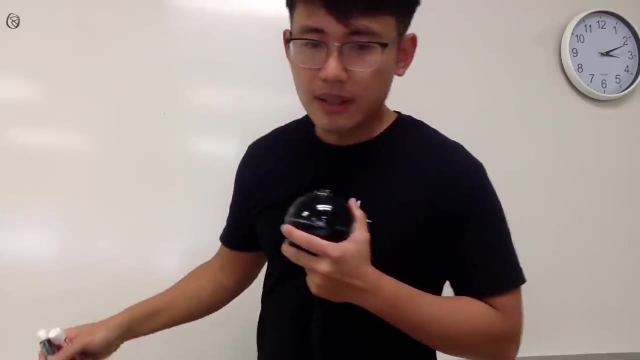 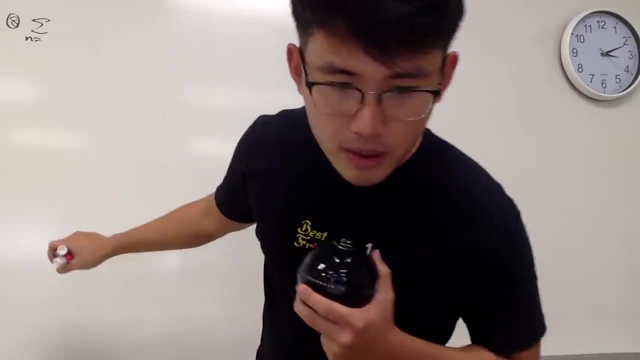 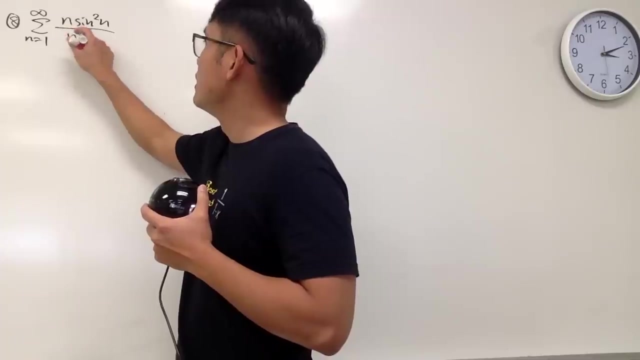 one day. Maybe you guys will bump into me on the street one day. Anyway, number 8 right here. Alright, number 8.. We have the sum, as n goes from 1 to infinity and n times sine squared, n over n to the third power. 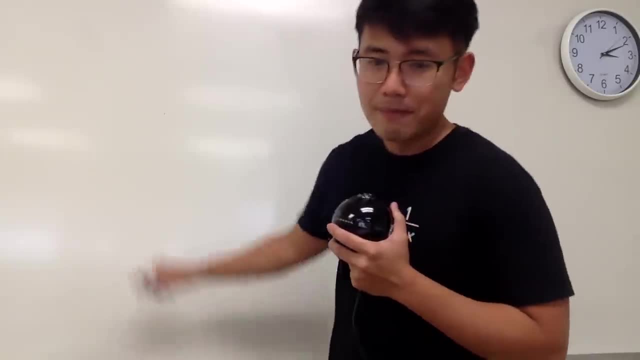 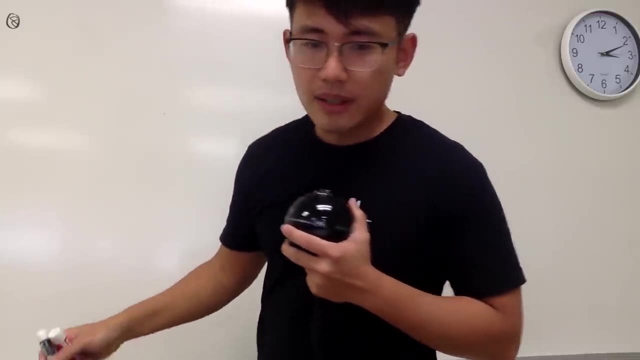 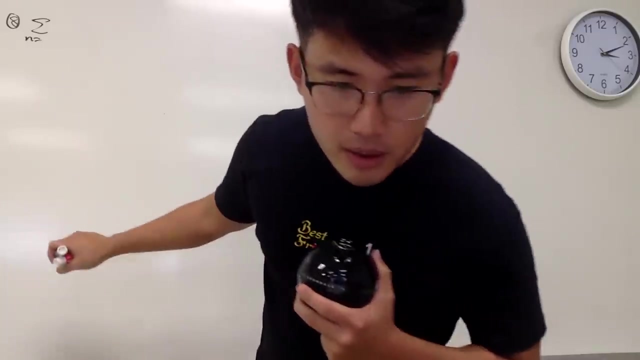 one day, you know, maybe you guys will bump into me on the street one day. Anyway, number 8, right here, Alright, number 8.. We have the sum as n goes from 1 to infinity and n times sine. 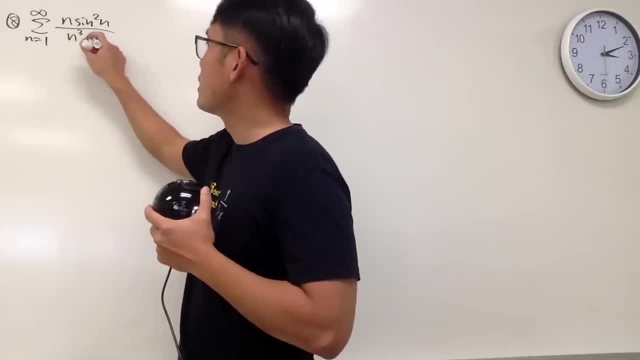 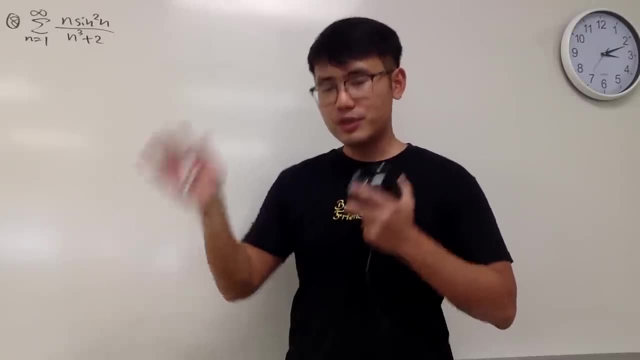 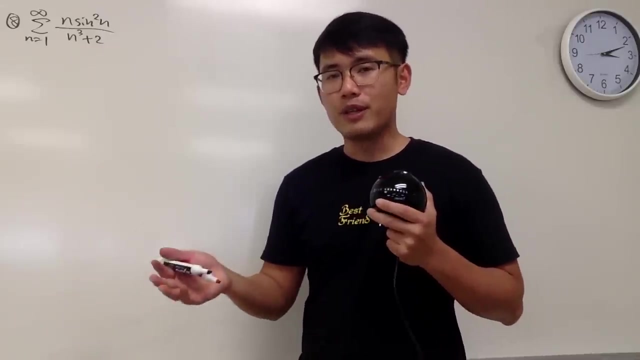 squared n over n to the third power plus 2.. Okay, here is the deal. Whenever you have sine cosine, just take the absolute value. Usually that will work out really nicely. And the reason is because, sine cosine, the maximum value for them is just. 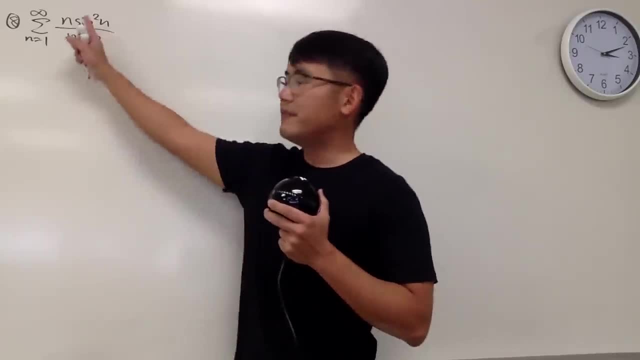 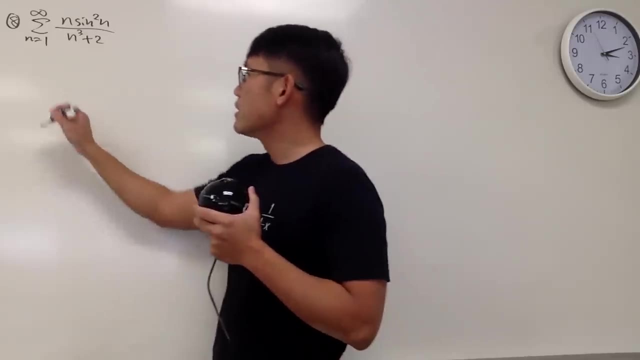 1,, even though here we have the square, And the idea is that, you see, in fact here everybody is positive, So we get to use the direct comparison test. So that's very nice. So now here we go. 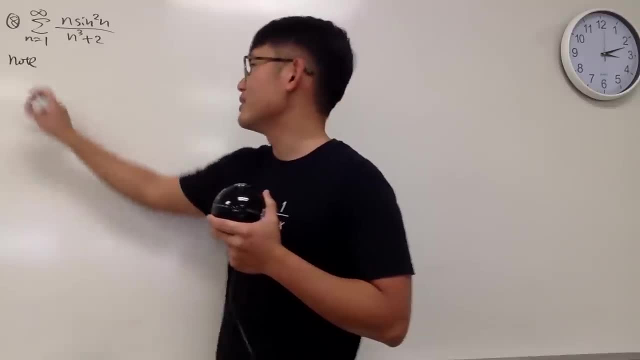 I'll just put down a note, We'll observe, I think, a note. I'll take a note on this Note and observe same thing. So we'll see that n goes from 1 to infinity. We take the absolute value. 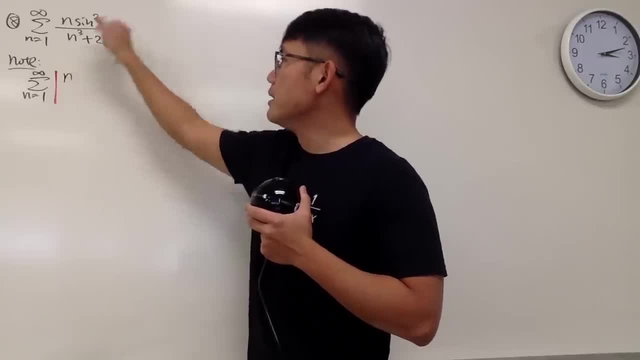 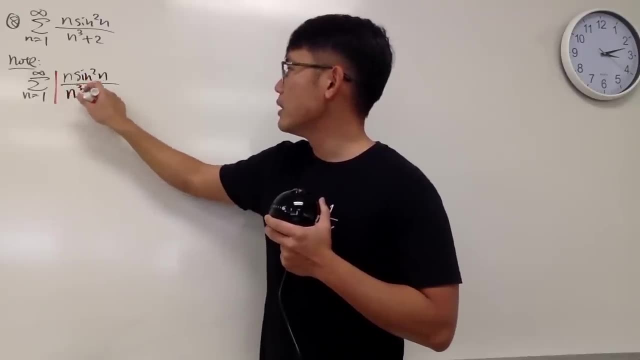 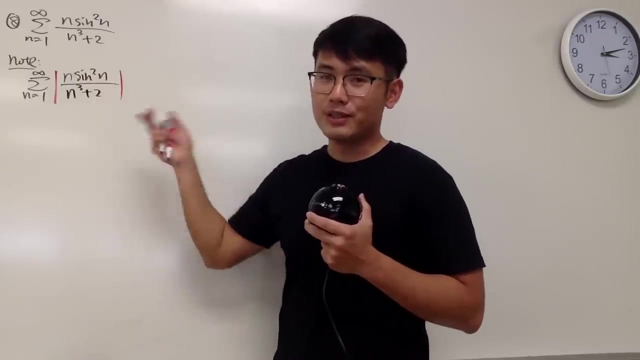 of this expression, n on the top, and then we have the sine squared, n over n to the third power, plus 2, like this, and then the absolute value, First thing. first, this right here becomes: we can say that less than or equal to 1. 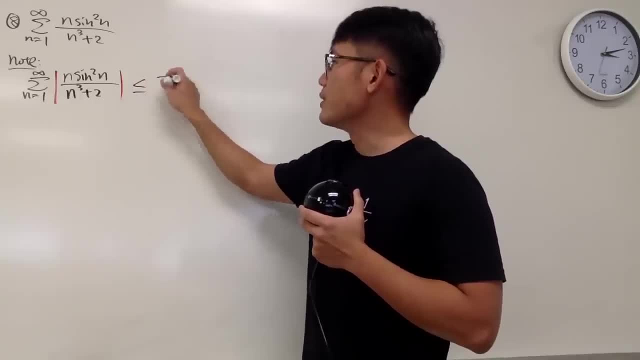 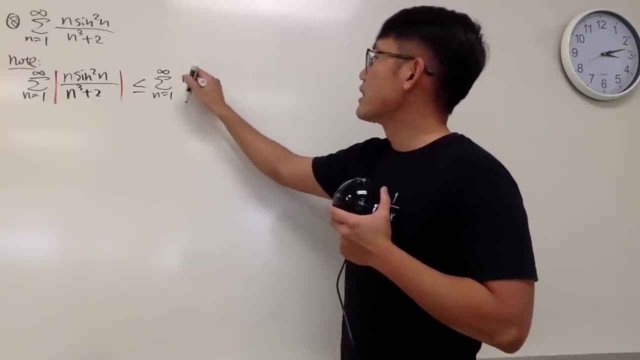 for the sine squared part. So we'll just write this down: This is less than or equal to the sum as n goes from 1 to infinity. This is you know. this is 1. now We have n times 1 over n to the third power. 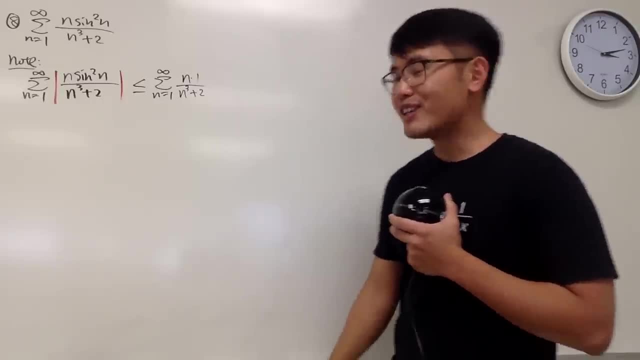 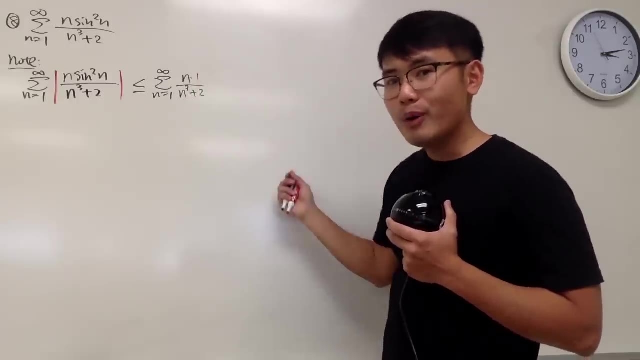 plus 2, like this. And now for the denominator. we are adding 2 to this. If I ignore the plus 2, the denominator is going to be smaller than the. the result will be bigger. So in other words, 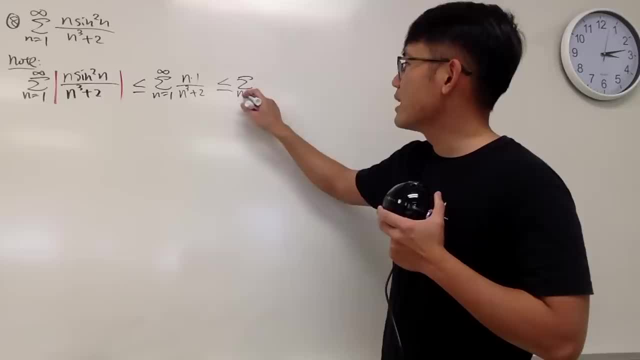 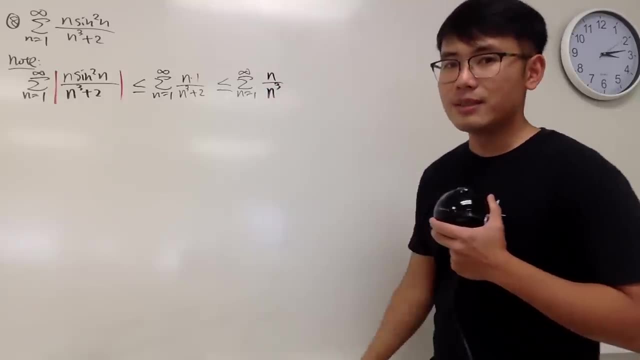 we can say this is less than or equal to the sum, as n goes from 1 to infinity. Just this over that n over n to the third power. Of course we can reduce that. This is the same as saying: and this is how you read the: 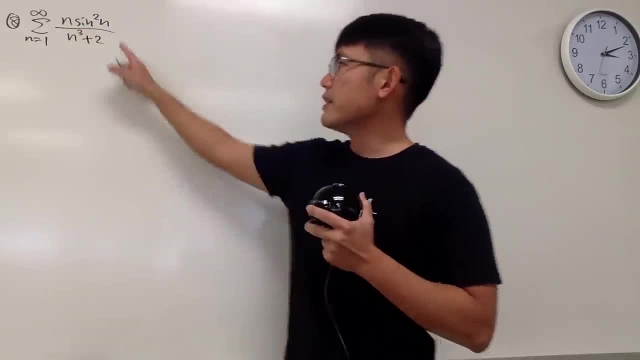 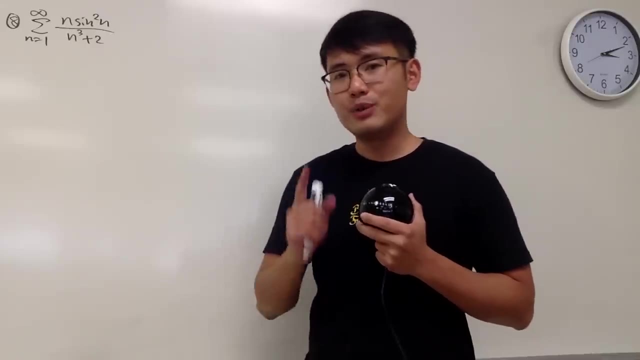 plus 2.. Okay, here is the deal: Whenever you have sine cosine, just take the absolute value. Usually that will work out really nicely. And the reason is because sine cosine, the maximum value for them is just 1, even though here we have the square. 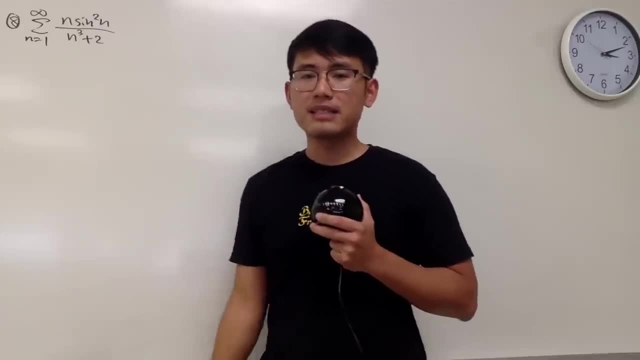 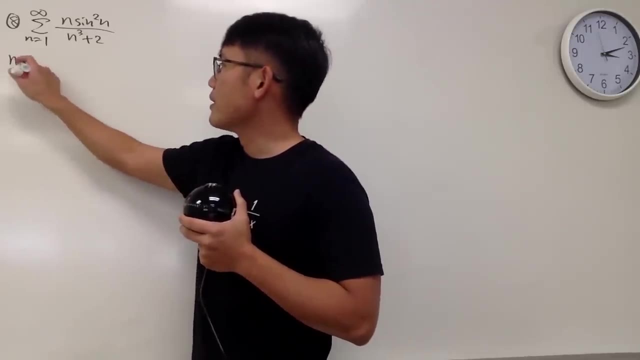 And the idea is that, you see, in fact here everybody is positive, So we get to use the direct comparison test. So that's very nice. So now here we go. I'll just put down a note, We'll observe. 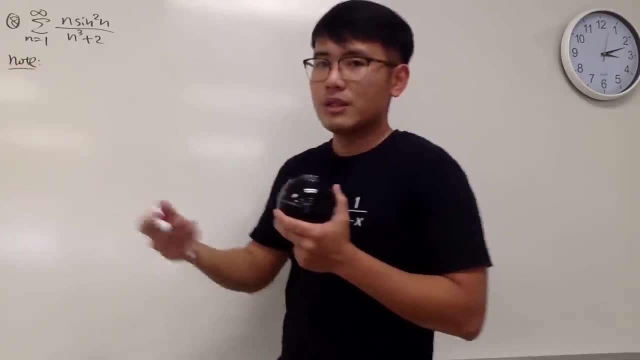 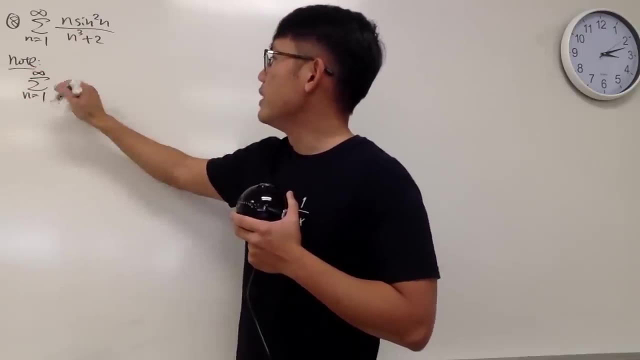 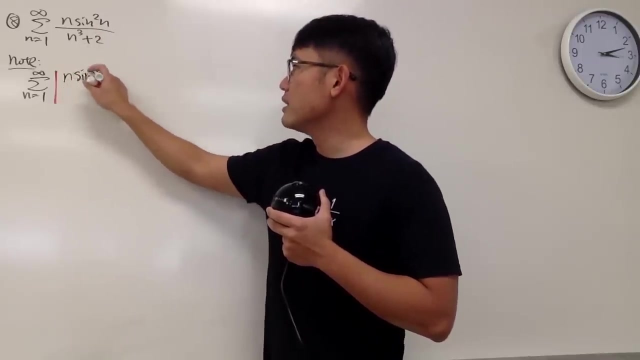 I think a note. I'll take a note on this Note and observe same thing. So we'll see that as n goes from 1 to infinity, we take the absolute value of this expression, n, on the top, and then we have the sine. 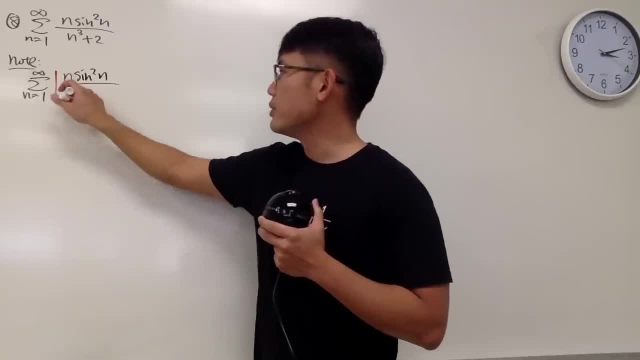 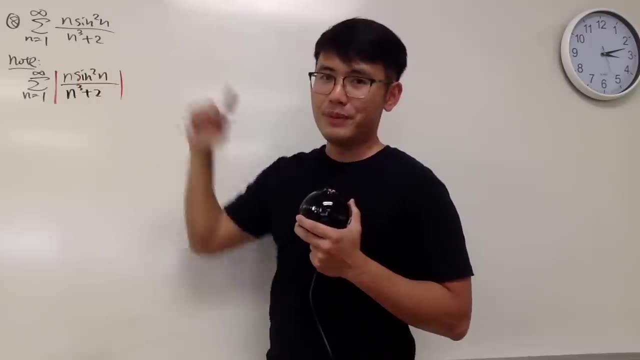 squared n over n to the third power plus 2, like this, And then the absolute value, First thing. first this right here becomes: we can say that's less than or equal to 1 for the sine squared part. So we'll just 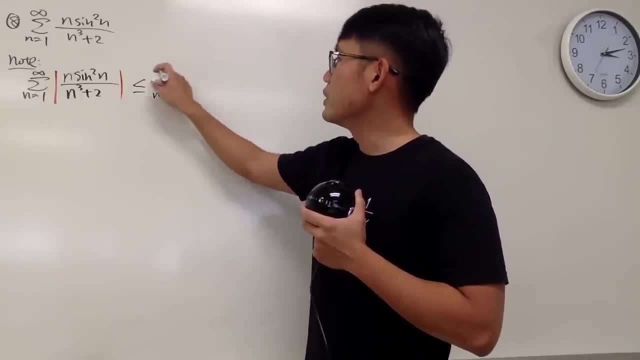 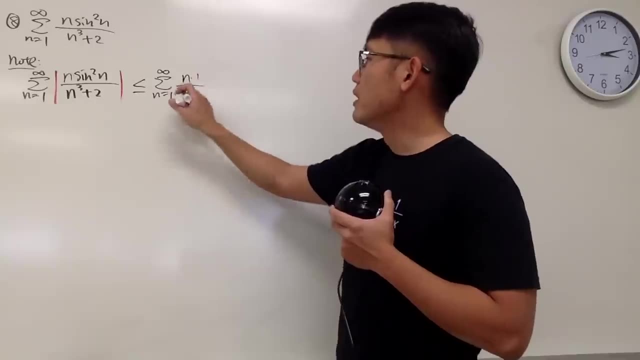 write this down. This is less than or equal to the sum, as n goes from 1 to infinity. This is, you know. replace it with 1. now We have n times 1 over n to the third power plus 2, like this: 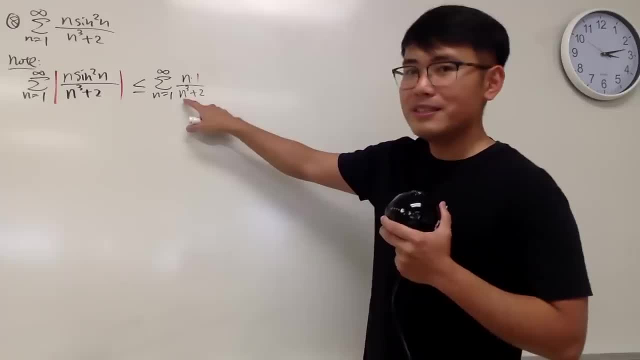 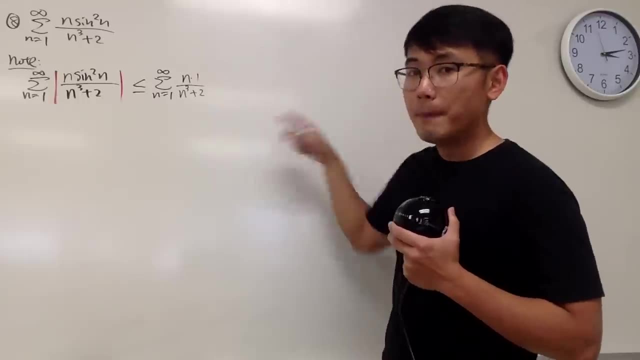 And now for the denominator. we are adding 2 to this. If I ignore the plus 2, the denominator is going to be smaller, then the result will be bigger. So in other words, we can say this is less than or equal to. 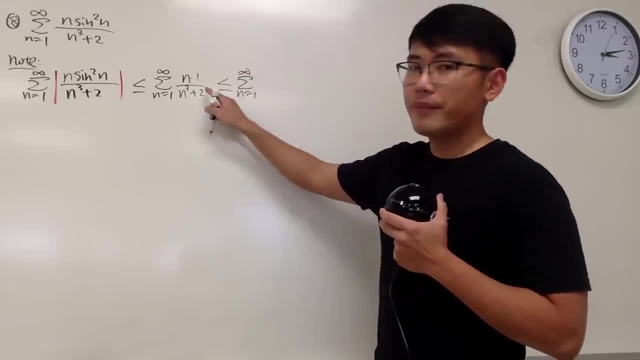 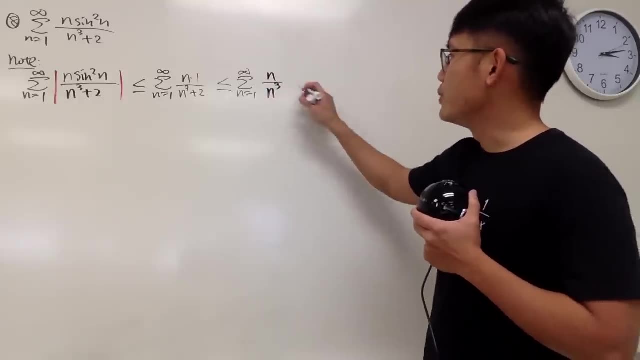 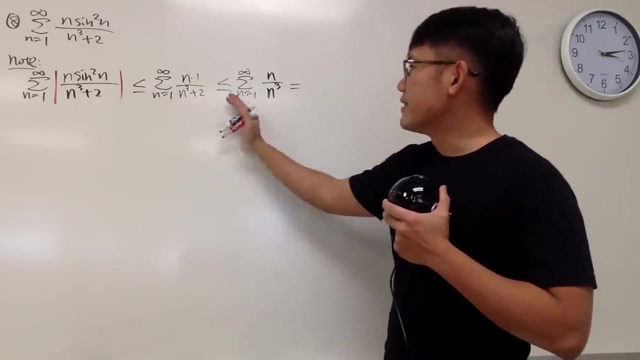 the sum as n goes from 1 to infinity, Because this over that n, over n to the third power. Of course we can reduce that. This is the same as saying: and this is how you read the inequality with the expression right here: This is less than that. 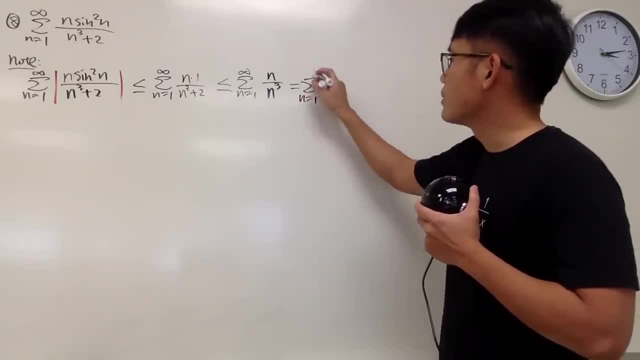 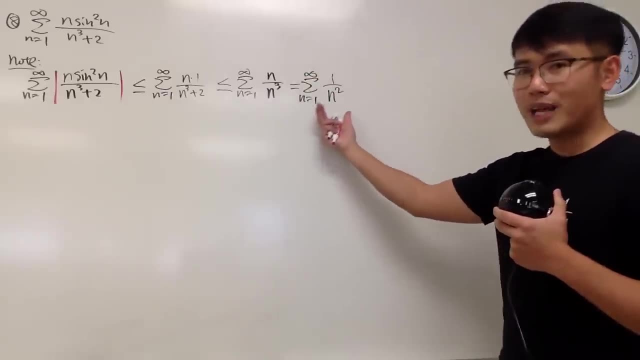 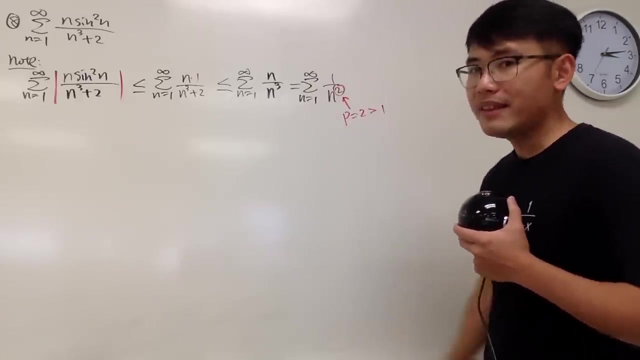 but this expression is equal to the sum as n goes from 1 to infinity, 1 over n. squared In another word, this is less than or equal to that right And of course this is great because we notice p is 2, which is greater than 1.. 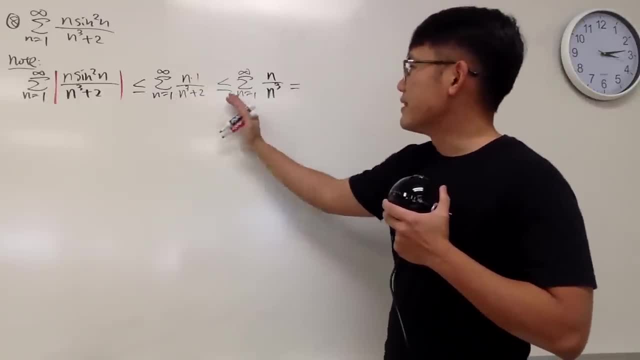 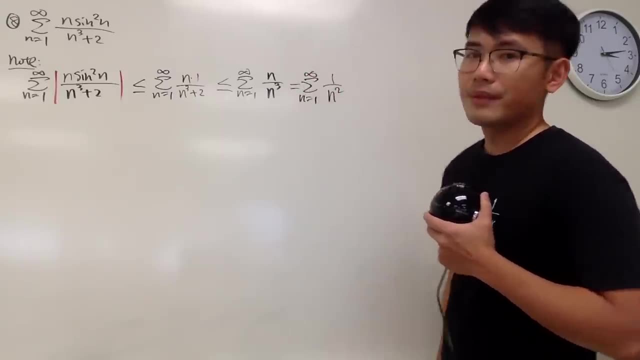 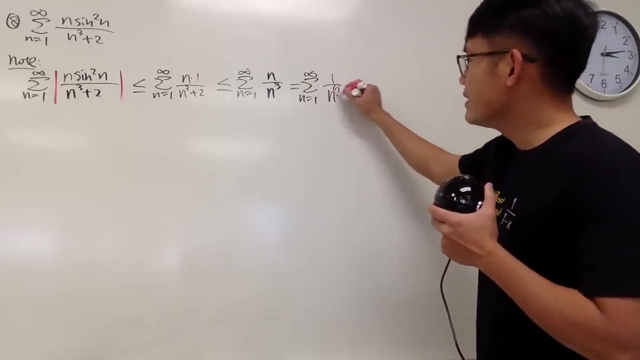 inequality with the expression right here. This is less than that, but this expression is equal to the sum as n goes from 1 to infinity. 1 over n. squared In another word, this is less than or equal to that right And of course, this is great. 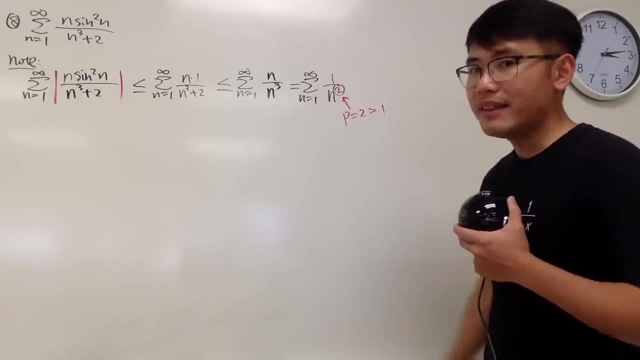 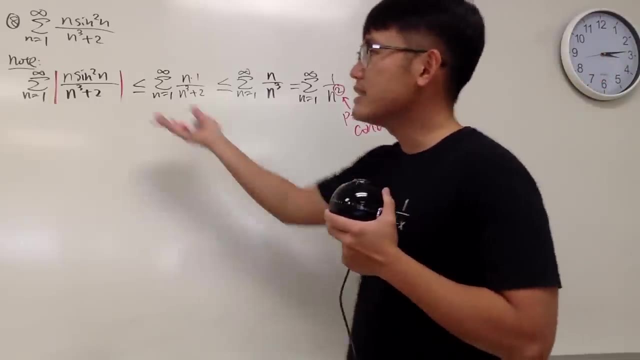 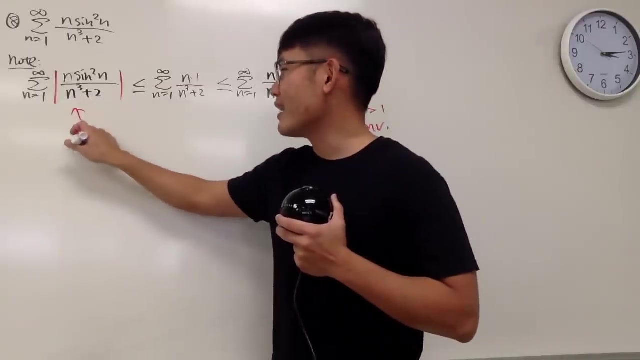 because we notice p is 2,, which is greater than 1, and this is a convergent p series. And the beauty is that this right here is less than a convergent. this right here is younger than a young person, so this right here is also young. 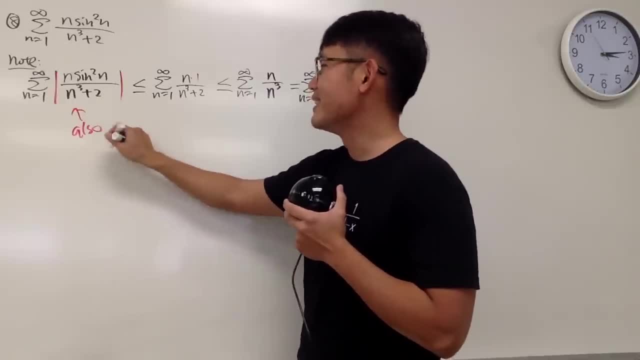 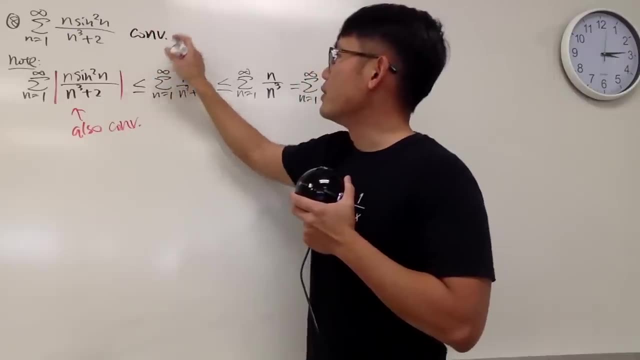 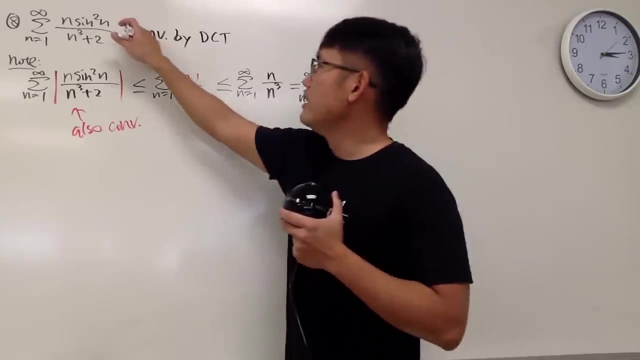 But of course we are talking about series, so we have to be serious. This is also convergent. So right here we will say this, right here, converges by the direct comparison test. And the truth is you can also say this is: 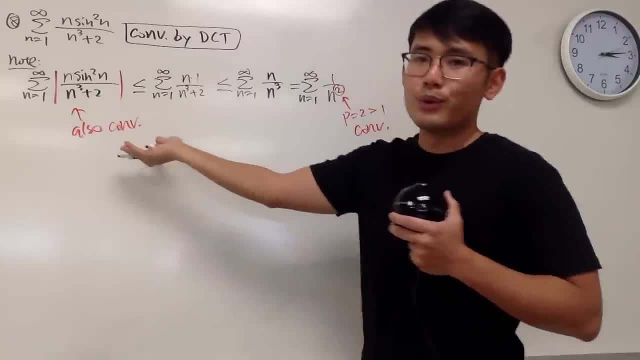 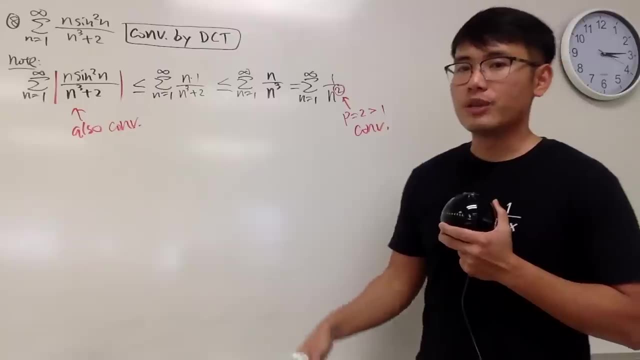 an absolute convergent because you took the absolute value of the terms. But you know, unless the question specifically asks you if it's absolute convergence or not, you don't really have to mention it. Absolute convergence implies it's a convergent. 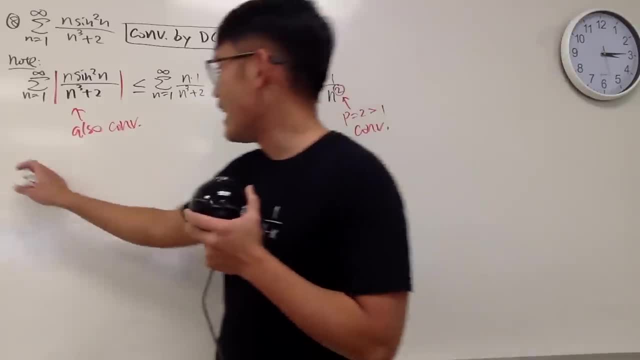 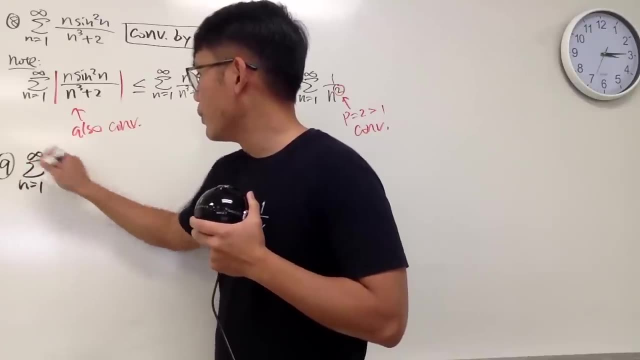 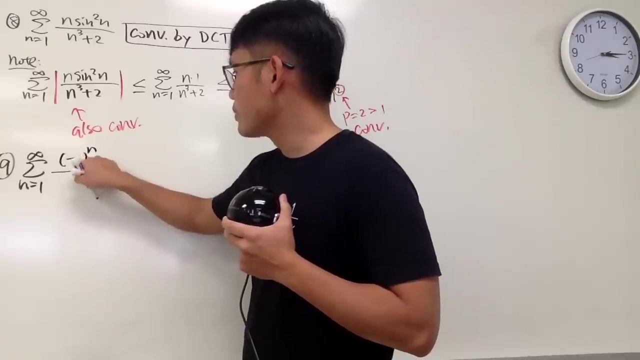 Anyway, this is it Now, number 9.. We have the sum as n goes from 1 to infinity. We have negative 1 to the nth power over square root of n plus 1. Like this. So here is the deal, This. 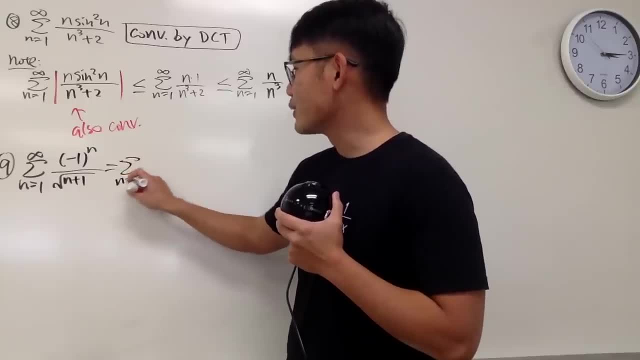 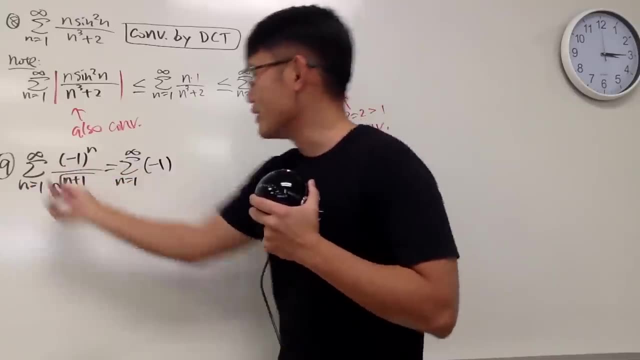 right here. let me just rewrite this as the sum as n goes from 1 to infinity. Let me put this in the front a little bit like this. You cannot take this all the way to the front, It's just like in the front of this part. Negative 1. 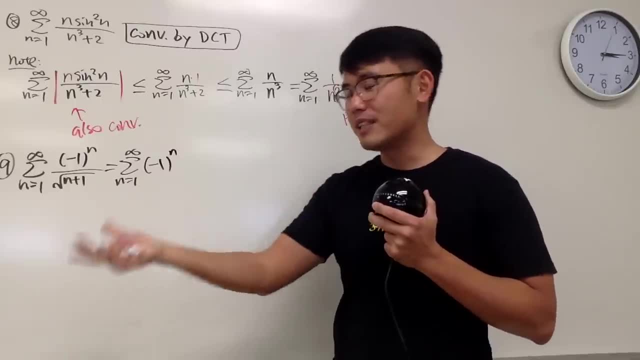 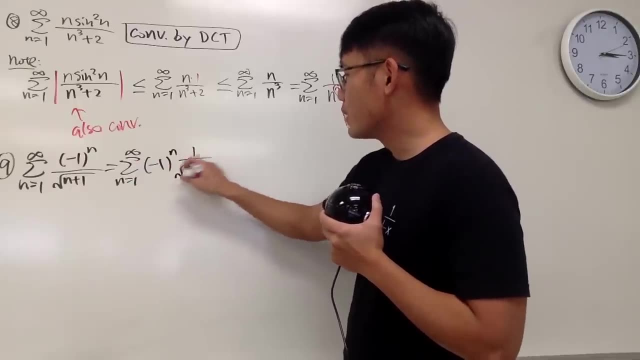 to the nth power, because this is the alternating part that gives the minus 1 plus 1 and so on, And start with 1, so minus 1 goes first, And then we have 1 over square root of n plus 1.. 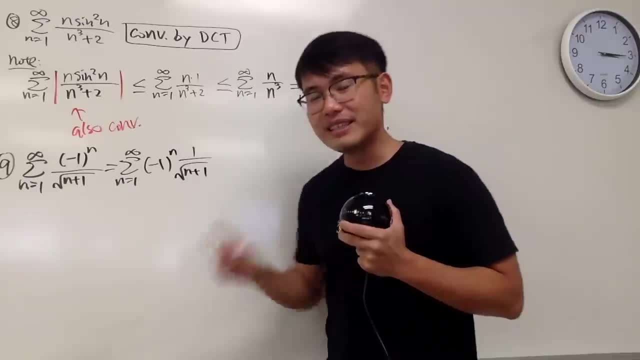 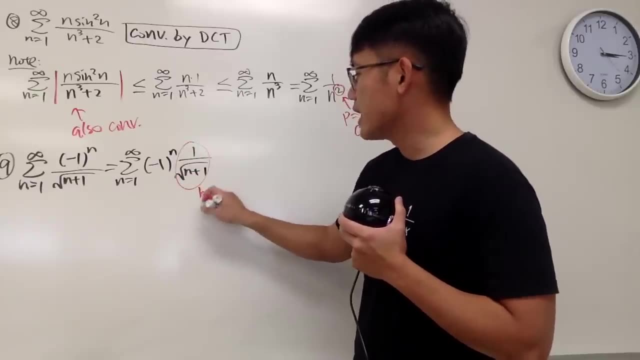 Like that: Right Now, this right here is an alternating series, And when you have an alternating series you will have to say, hey, this right here is our bn And we have to do two checks. So here we go. 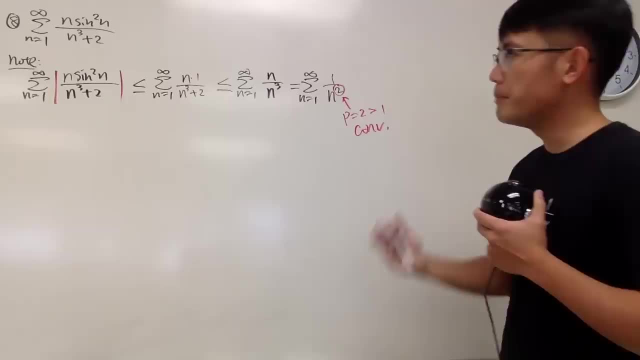 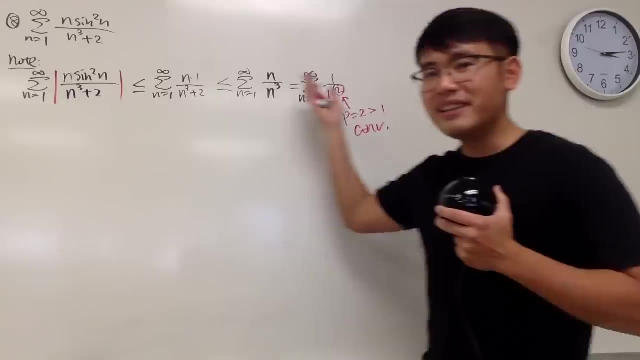 And this is a convergent p series And the beauty is that this right here is less than a convergent. This right here is younger than a young person, So this right here is also young, But of course we are talking about series. 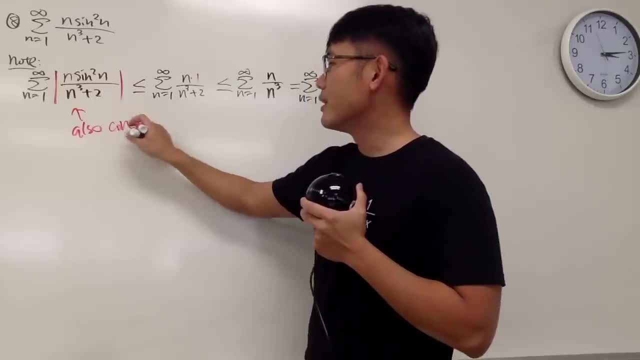 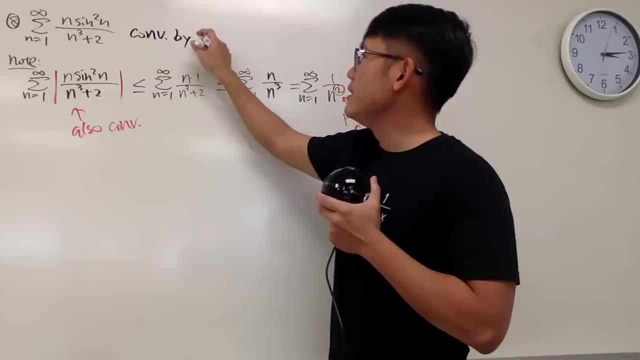 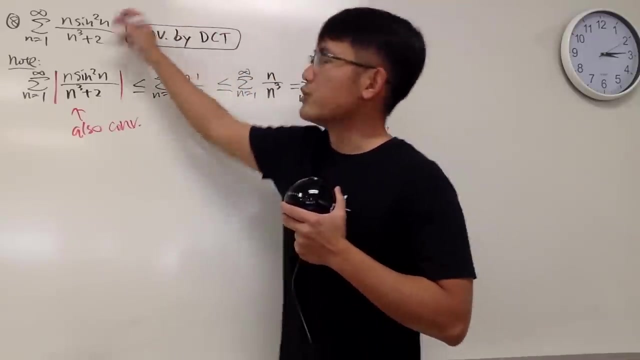 so we have to be serious. This is also convergent. So right here we will say this, right here: converges by the direct, constant test. And the truth is you can also say this is absolute convergent because you took the absolute value of the 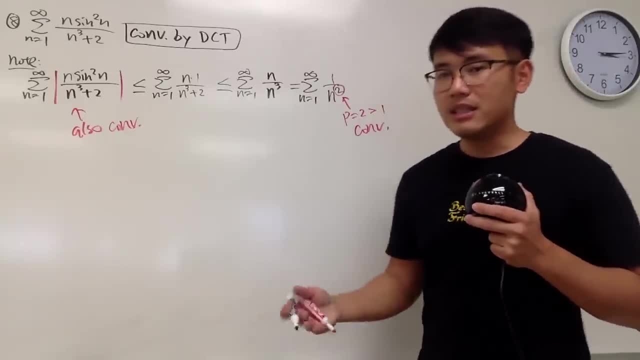 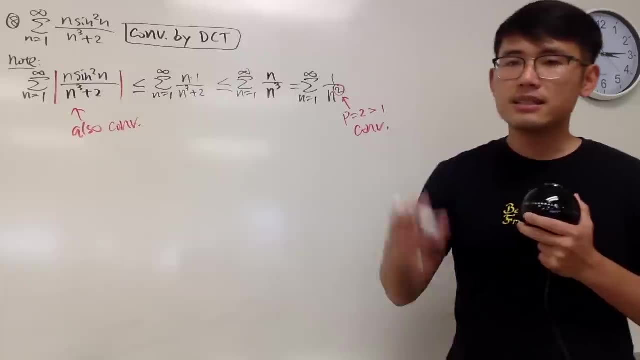 terms. But you know, unless the question specifically asks you if it's absolute convergence or not, you don't really have to mention it. Absolute convergence implies it's a convergent. Anyway, this is it Now number 9.. 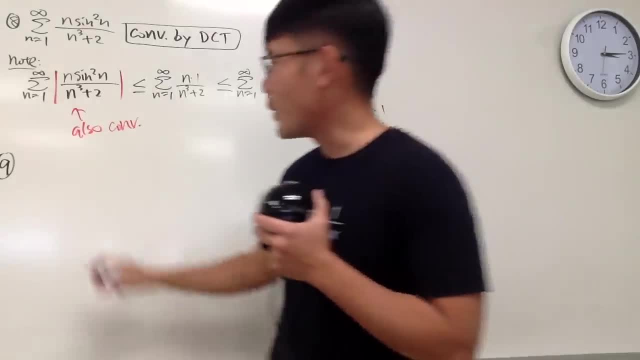 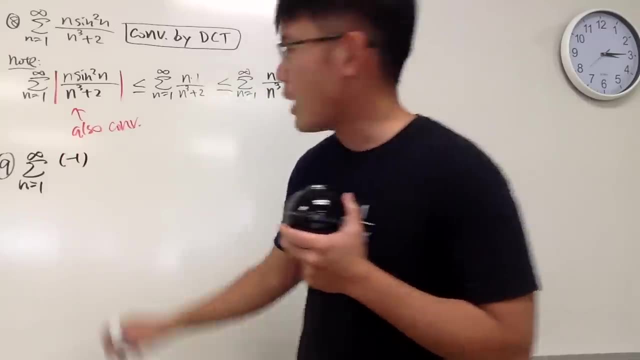 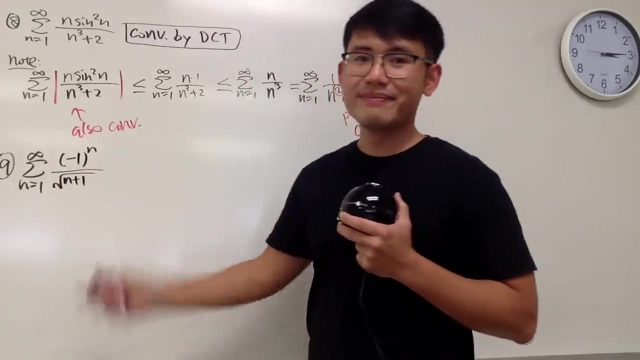 We have the sum as n goes from 1 to infinity. We have negative 1 to the nth power over square root of n plus 1.. Like this. So here is the deal, This right here. let me just rewrite this as the sum as n goes from 1. 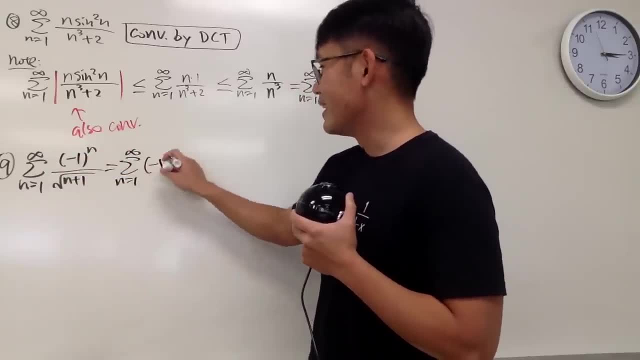 to infinity. Let me put this in the front a little bit like this: You cannot take this all the way to the front. It's just like in the front of this part: Negative 1 to the nth power, because this is the. 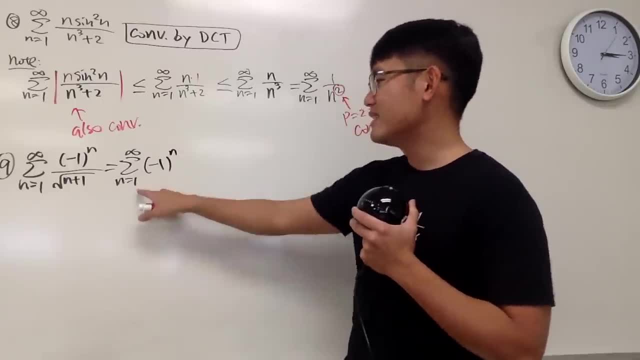 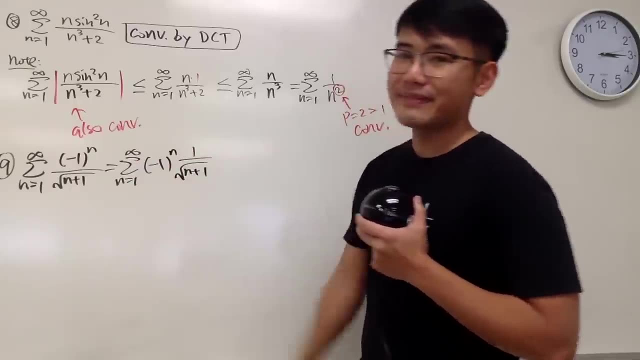 alternating part that gives you the minus 1 plus 1.. And so on. n starts with 1, so minus 1 goes first, And then we have 1 over square root of n plus 1.. Like that, Right Now, this right here is an alternating. 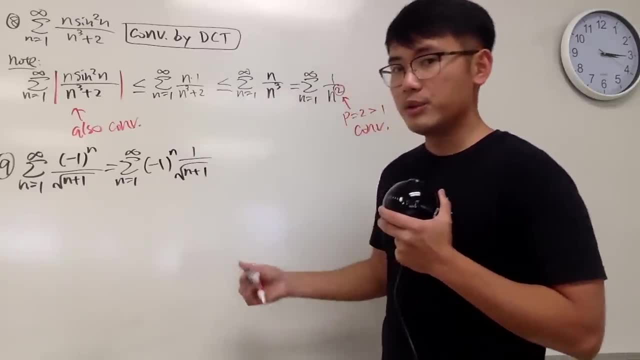 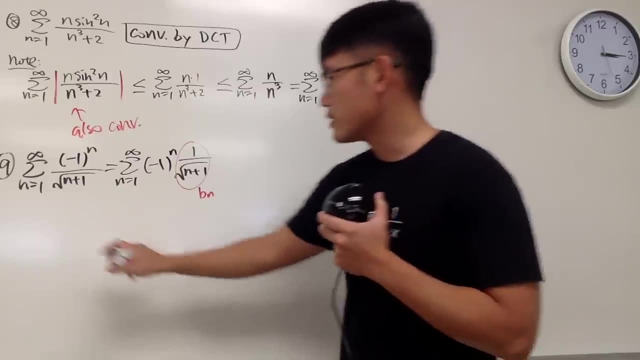 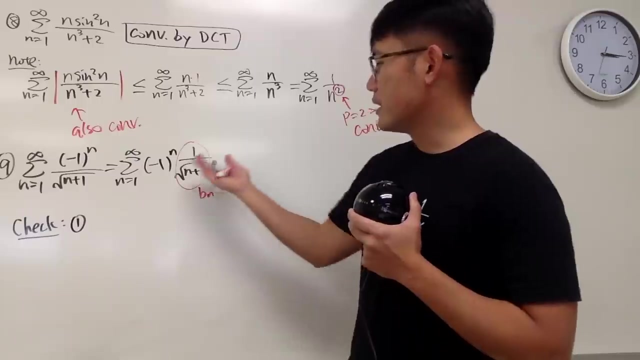 series, And when you have an alternating series you will have to say, hey, this right here is our bn And we have to do two checks. So here we go, Check number 1.. Well, the bn goes to 0.. 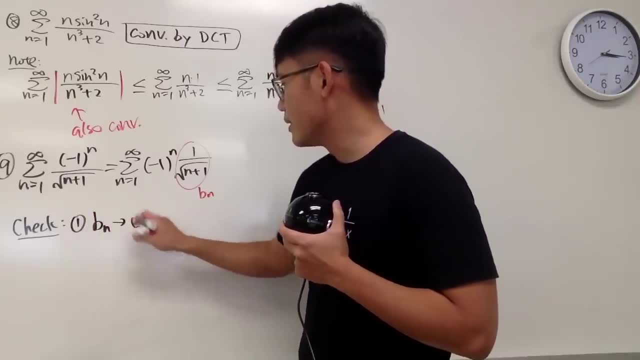 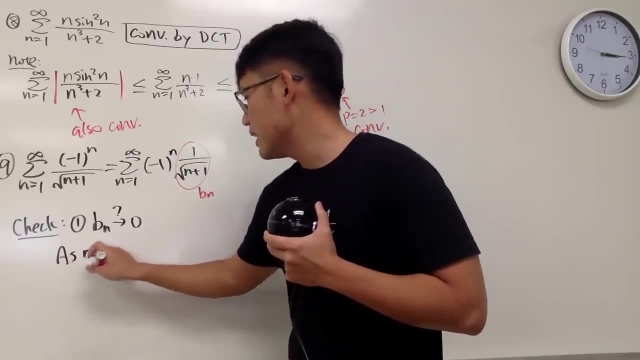 Let me just put it down. Does bn go to 0? Like this? I don't know. yet That is the first check, So I'll just put this down. As n goes to infinity, bn is 1 over square root of n plus 1.. 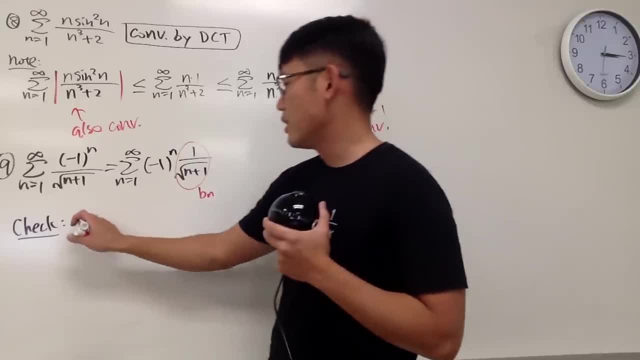 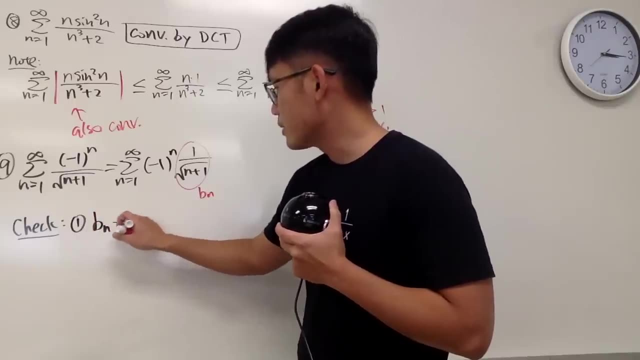 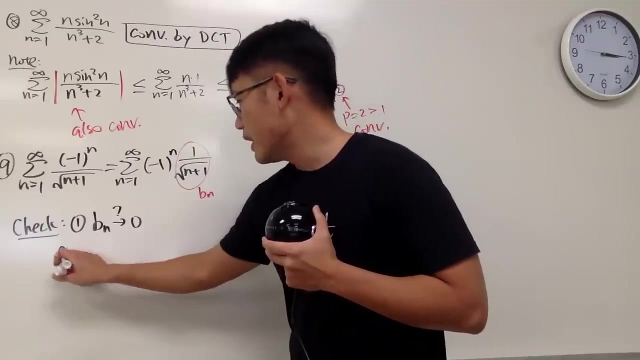 Check number 1.. Well, does bn go to 0?? Let me just put it down. Does bn go to 0? Like this? I don't know yet. That's the first check, So I'll just put this down. 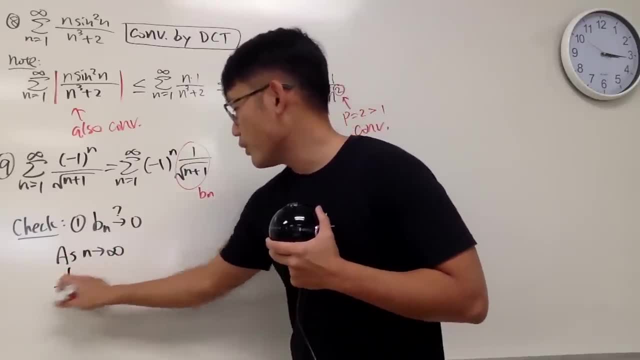 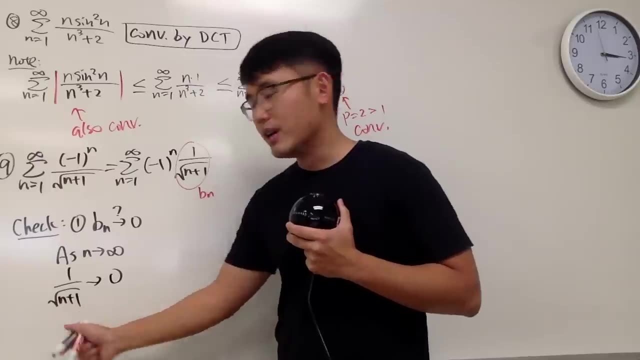 As n goes to infinity, bn is 1 over square root of n plus 1.. Does this approach 0?? Yes, it does. You can just put infinity down right here, So you do have the 1 over square root of infinity plus. 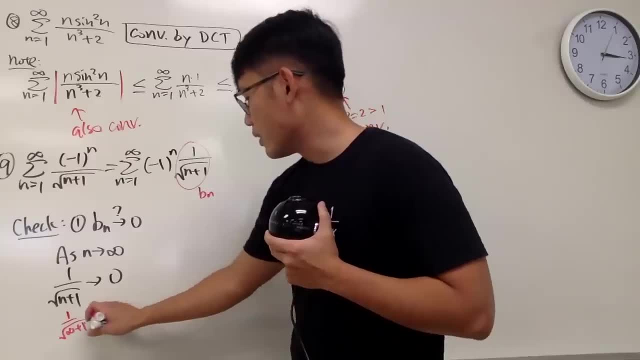 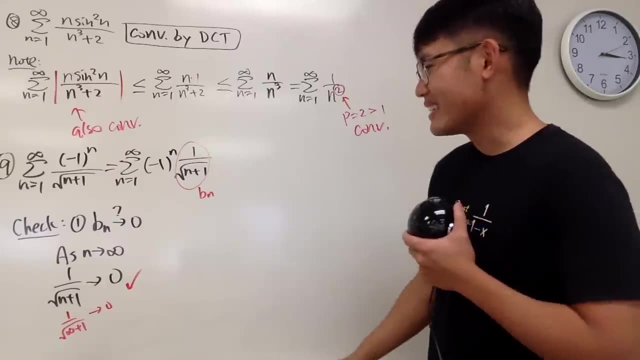 1. So this is pretty clear that it does approach 0. So you can just put a check mark to indicate that you've really checked it. So just do some work to indicate that, or you have to measure it, Number 2.. 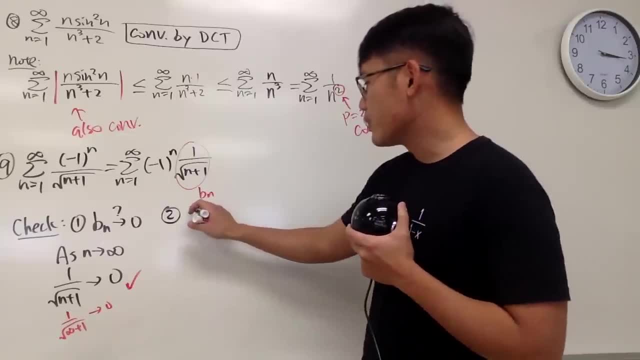 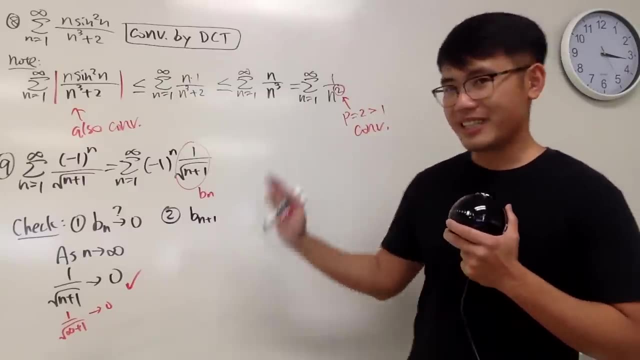 You have to make sure that bn is a decreasing sequence. So in other words, we have to see if bn plus 1, namely the next term, is it smaller than the current term? So I'll put down less than or equal to, less than or equal to, like this: 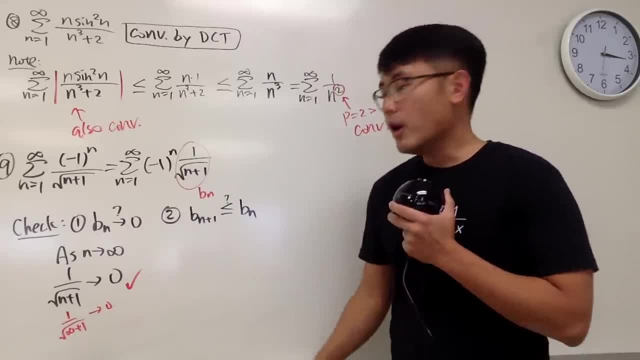 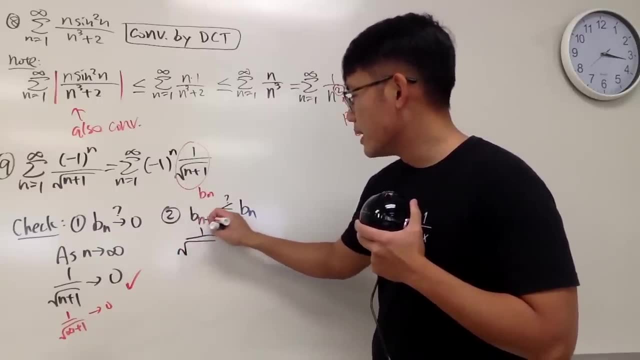 bn, And again, we don't know yet. Well, bn is this? so in this case we will get 1 over square root. I will just have to place the n plus 1 into this n, So we will have n plus 1. 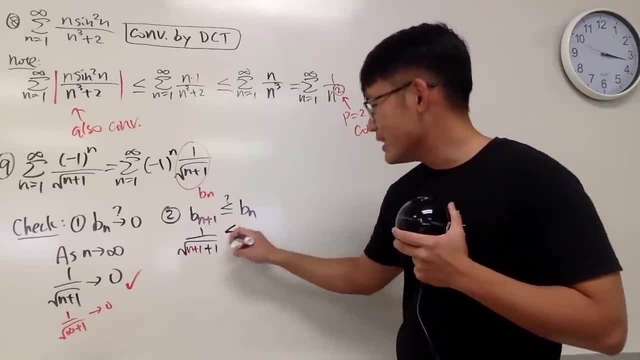 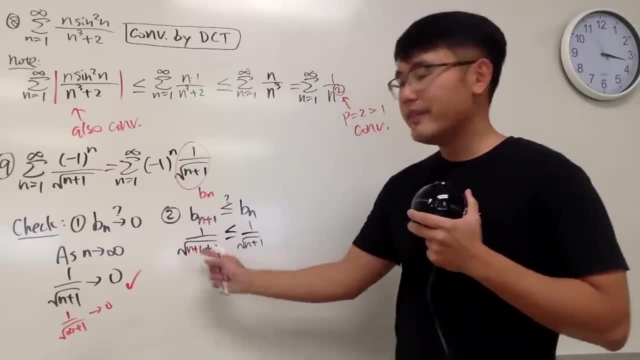 and n plus 1.. And do we get this bn less than or equal to 1 over square root of n plus 1? Of course it does, because right here the denominator is again bigger. That means the whole thing is smaller than that. So you can just say: 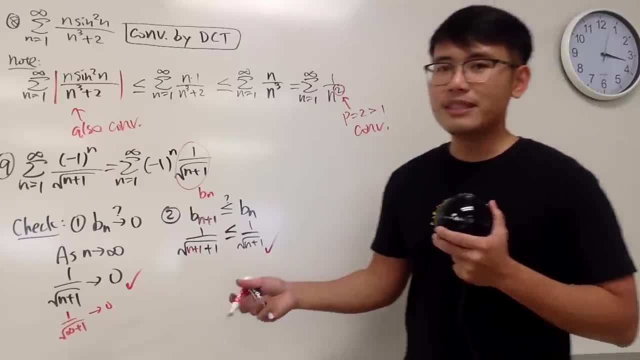 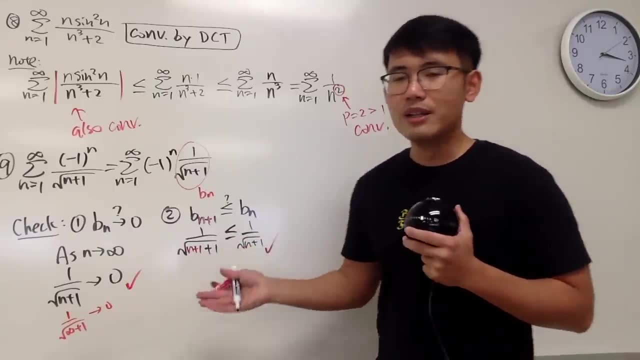 checks. Okay And seriously, I have seen a lot of students they just put down whatever they think that they have to put down and then just put down check marks Without really sure about what's going on. So you really have to give some reason. 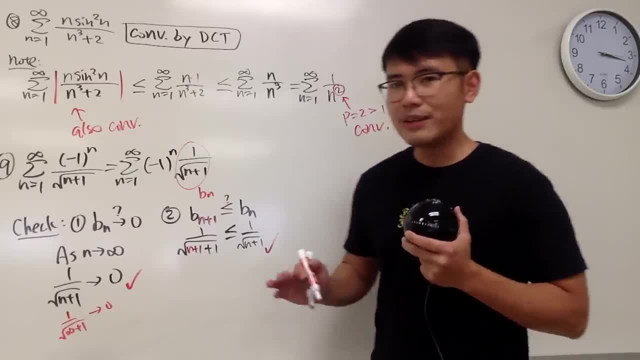 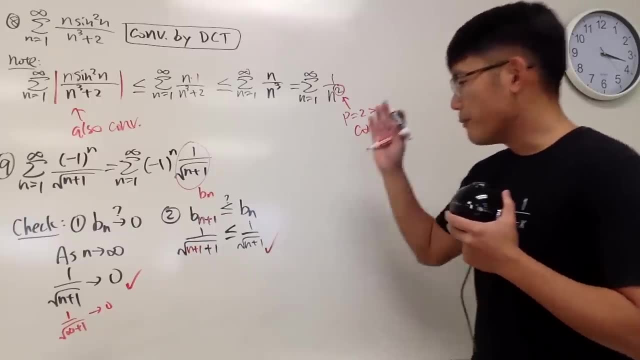 to yourself, Not just put down a check mark. okay, You really have to be sure you know what's happening, because you are technically writing proofs for all these kinds of questions. Alright, so this is it. These two satisfied it, So we can say that the original. 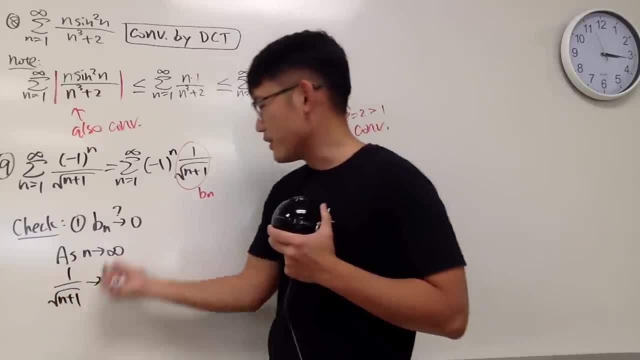 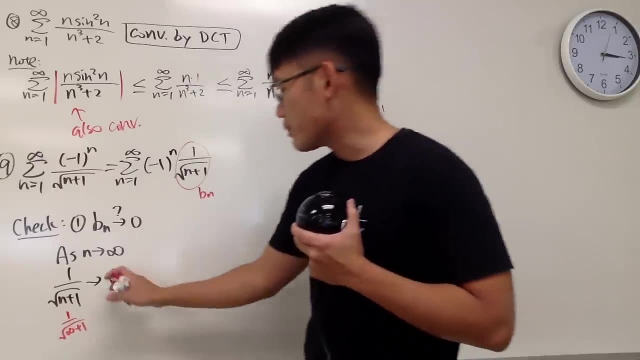 Does this approach 0?? Yes, it does. You can just put infinity down right here, So you do have the 1 over square root of infinity plus 1.. So this is pretty clear that it does approach 0. So you can just put a check mark. 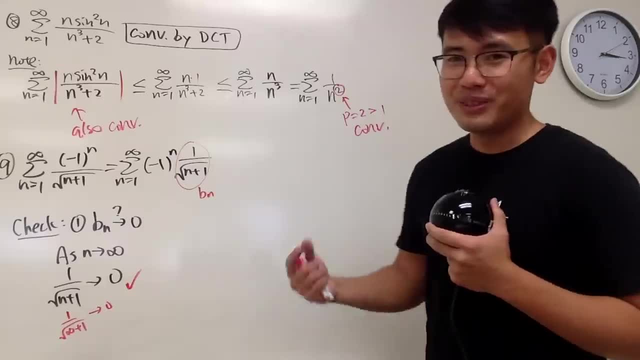 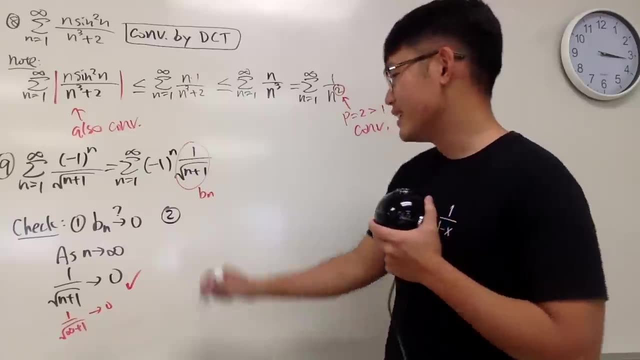 to indicate that you've really checked it. Okay, So just do some work to indicate that where you have to measure it, Number 2. You have to make sure that bn is a decreasing sequence. So, in another word, we have to see if bn plus. 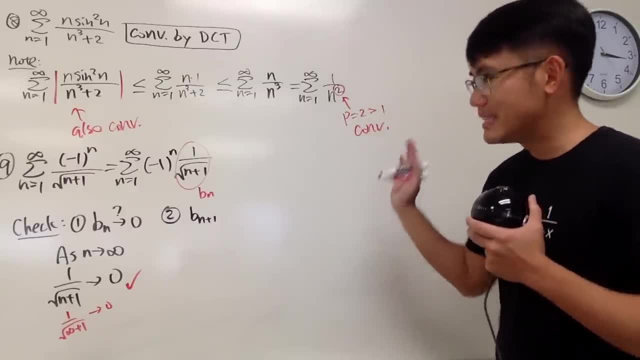 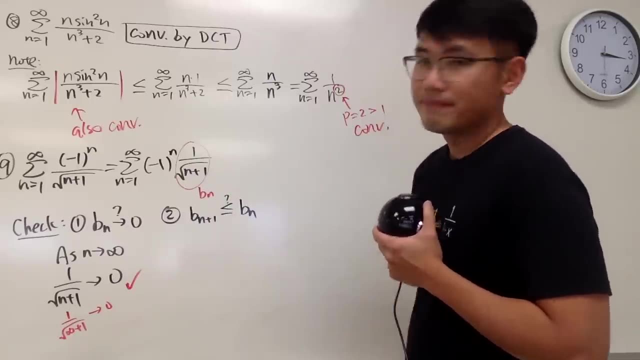 1, namely the next term. is it smaller than the current term? So I'll put down less than or equal to less than or equal to, like this bn, And again, we don't know yet. Well, bn is this. So in this case, 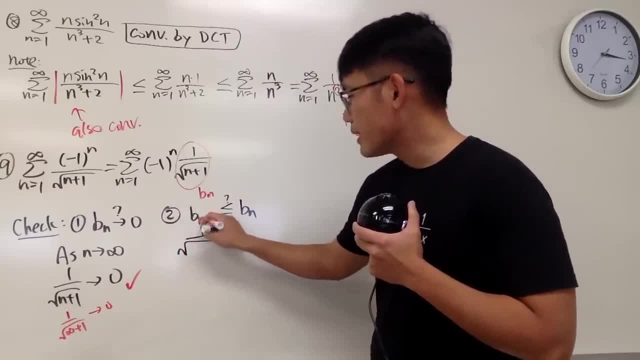 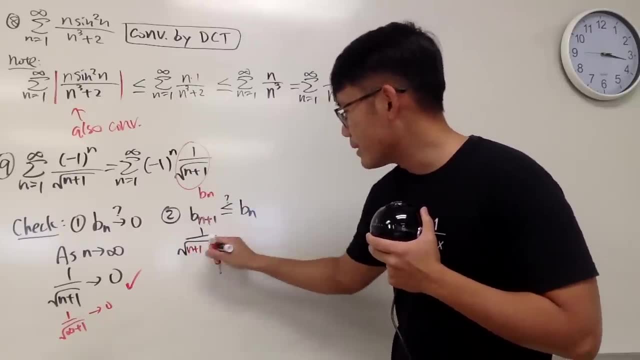 we'll get 1 over square root. I will just have to place the n plus 1 into this n, So we will have n plus 1 and n plus 1.. And do we get this bn less than or equal to 1 over square root of n? 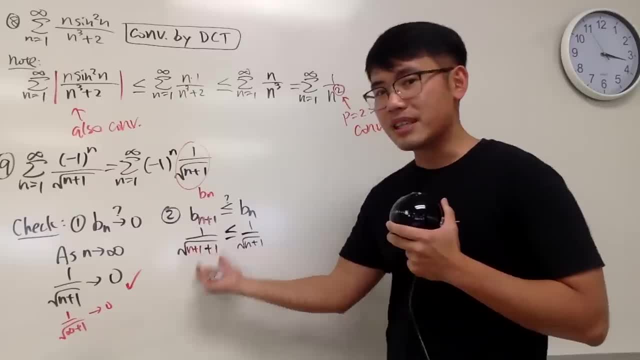 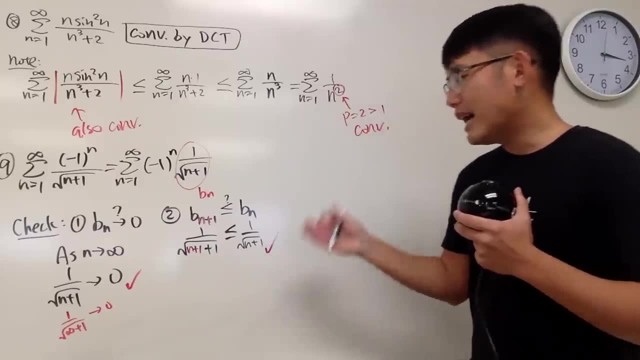 plus 1?? Of course it does, because right here the denominator is again bigger. That means the whole thing is smaller than that. So you can just say: checks Okay. And seriously, I have seen a lot of students. they just put down whatever they think. 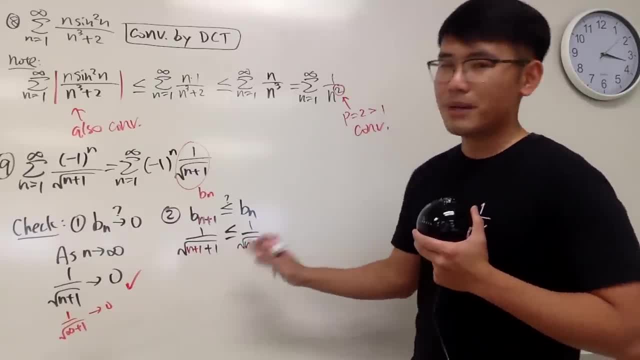 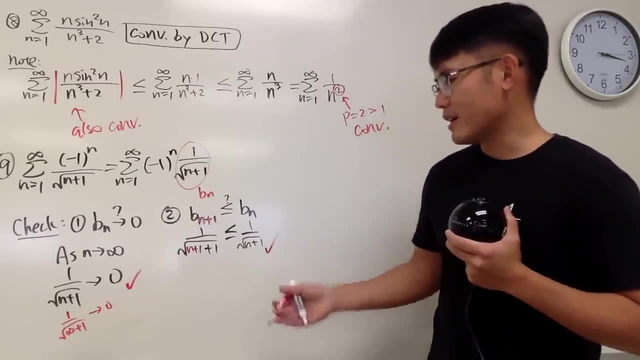 that they have to put down, and then just put down a check mark without really sure about what's going on. So you really have to give some reason to yourself, Not just put down a check mark, okay. You really have to be sure you know what's happening. 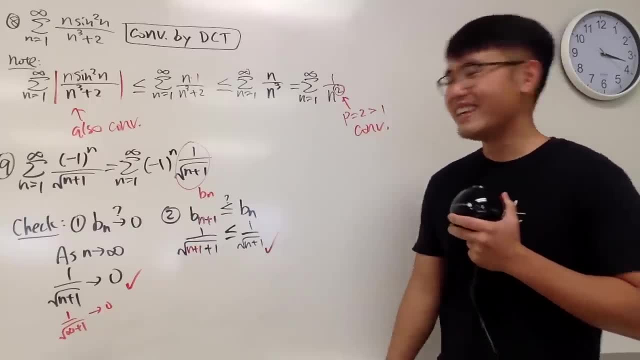 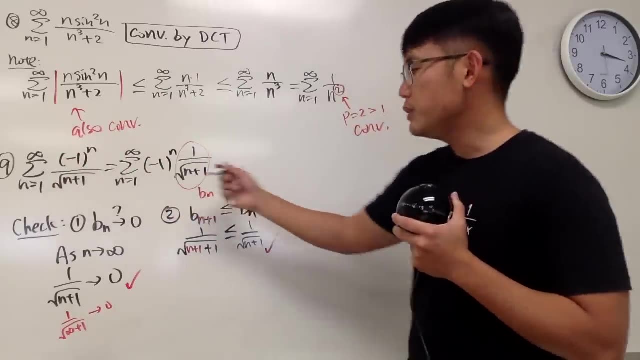 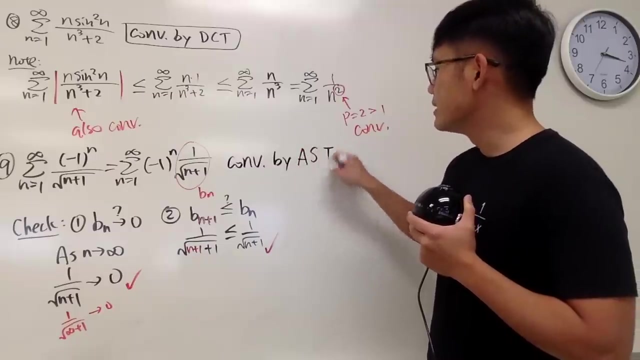 because you are technically writing proofs for all these kind of questions. Alright, so this is it. These two satisfied it. So we can say that the original series right here converges by the alternating series test, Right By the alternating series test. 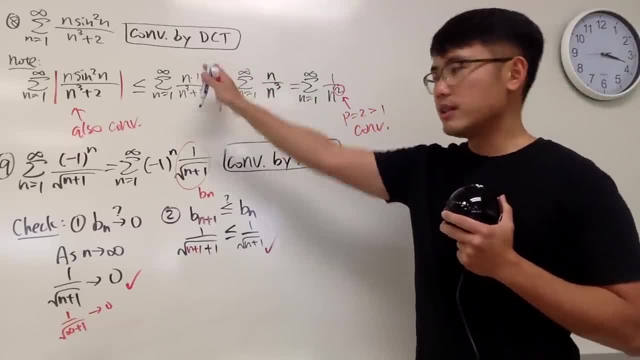 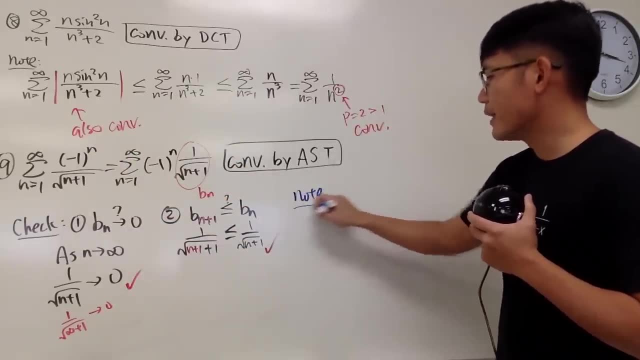 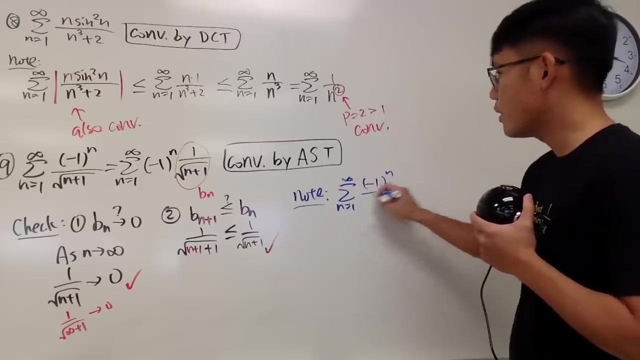 Okay, since we talked about the absolute convergence earlier, let's also mention this real quick. Let me just tell you guys that this right here, though note right, This right here- the sum as n goes from 1 to infinity of negative, 1 to the nth power over. 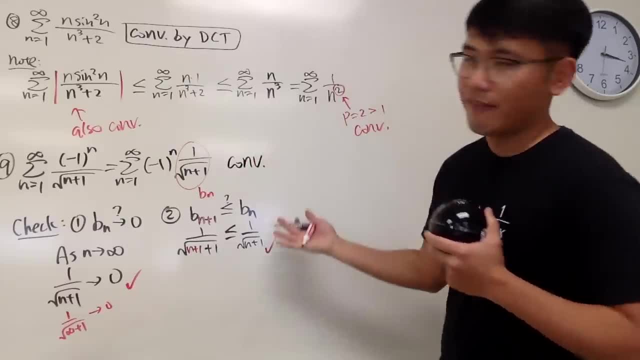 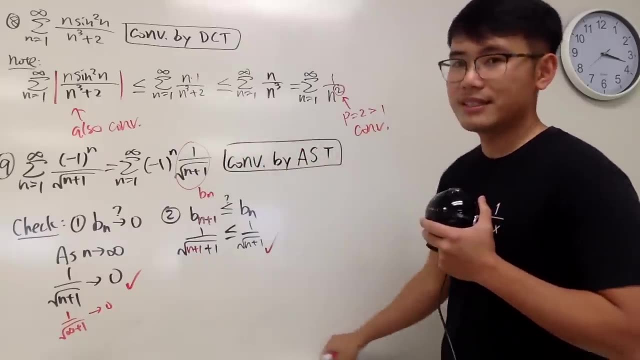 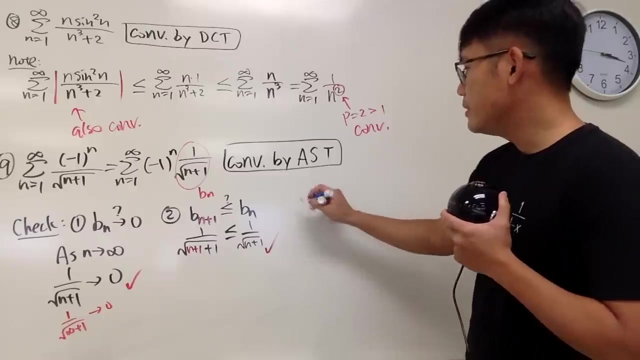 series right here converges by the alternating series test. Right By the alternating series test. Okay, since we talked about the absolute convergence earlier, let's also mention this real quick. Let me just tell you guys that this right here, though note. 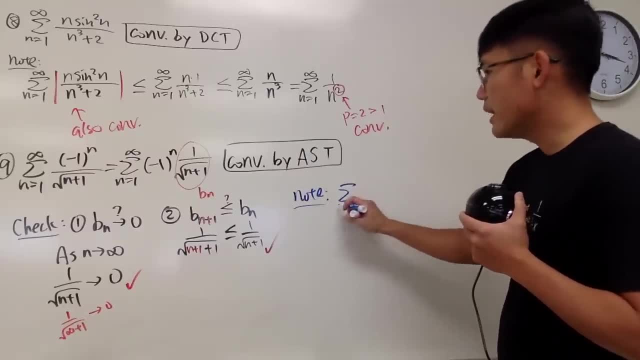 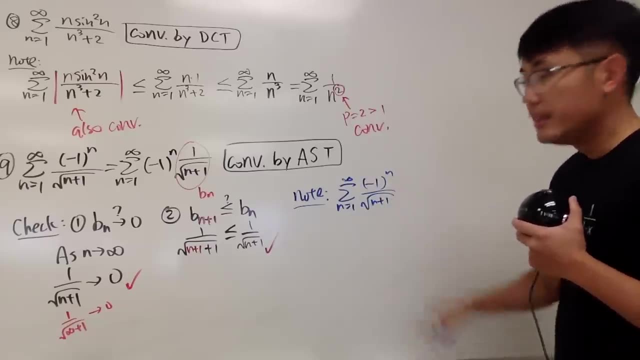 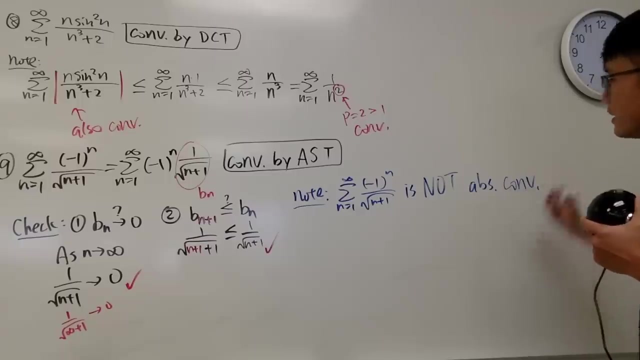 right. This, right here, the sum as n goes from 1 to infinity of negative, 1 to the nth power over square root of n plus 1.. This, right here, is not absolutely convergent. It does not converge absolutely Why? Because, if you check, 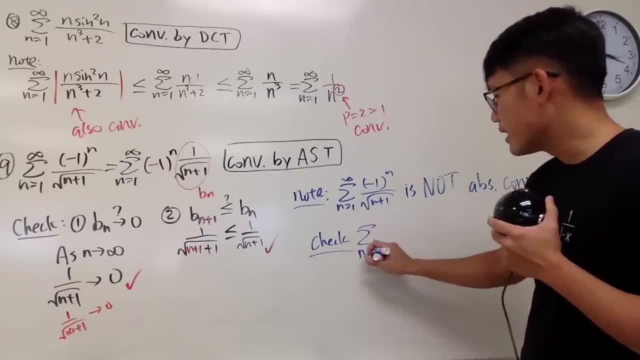 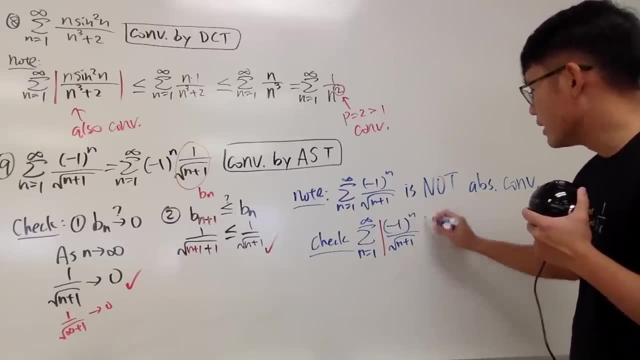 the limit, sorry, not the limit. the sum as n goes from 1 to infinity. if you take the absolute value of this negative 1 to the nth power over square root of n plus 1, like this: Well, this: 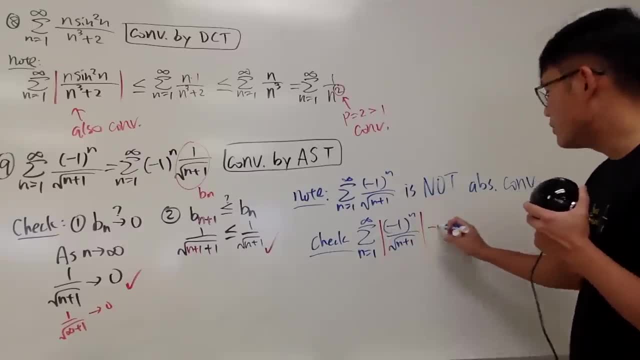 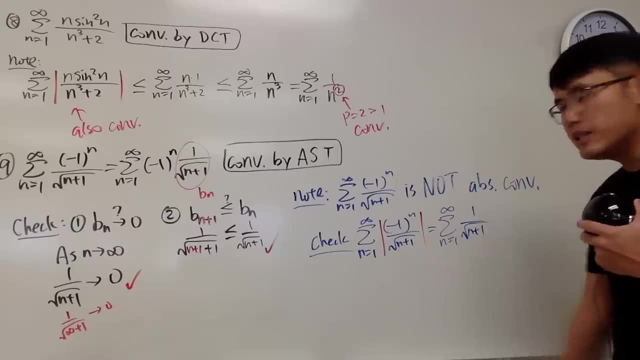 right here is just 1.. Negative 1 to whatever power you have, the absolute value everybody becomes 1.. So this is just n goes from 1 to infinity of 1 over square root of n plus 1.. And you see the absolute value version. 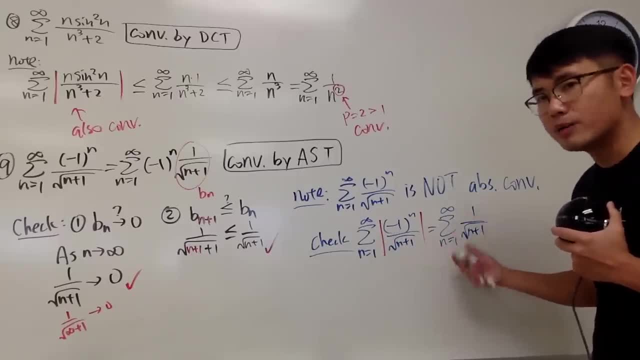 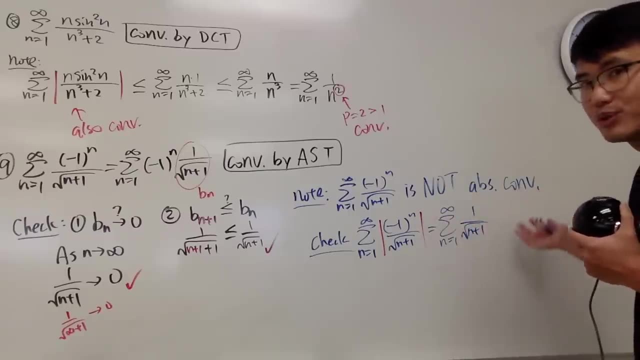 of this, you have pretty much an n to the 1 half power if you ignore that, And you can do some limit comparison test if you would like. Right, So you know, you can just do the things. This right here diverges. 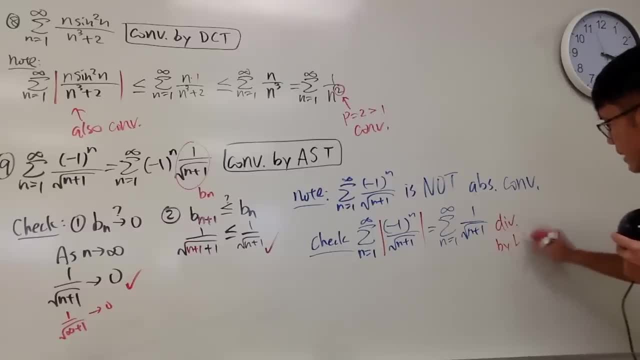 You can do it by limit comparison test with the sum, as n goes from 1 to infinity, of the square root of n. like this, Because here the p is 1 half, Which is less than 1.. Less than or equal to 1.. 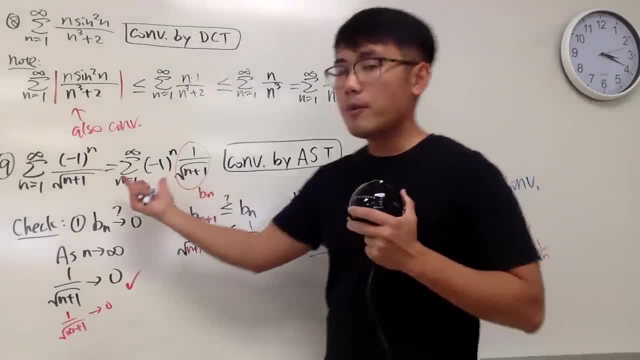 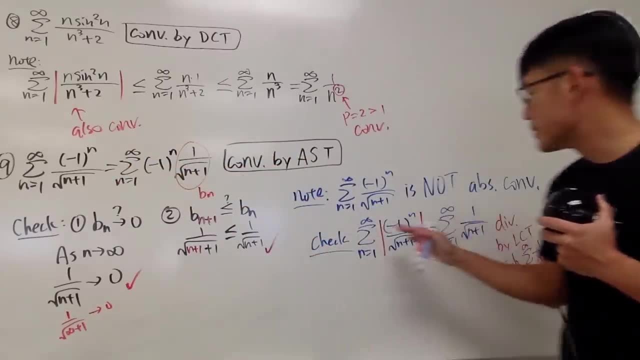 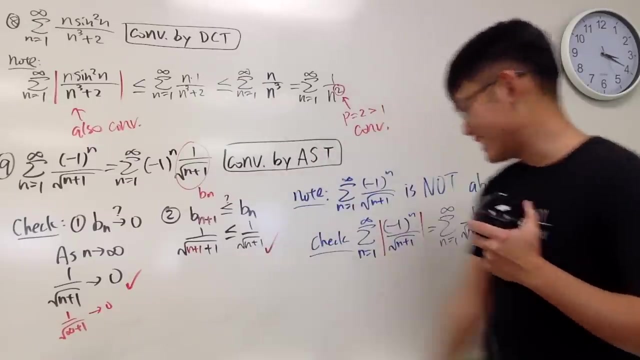 So it diverges. So this right here will be an example of a series that is a convergent, but it's not an absolute convergent, And in this case we say this: right here is a conditional convergent series. Right, That's number 9.. 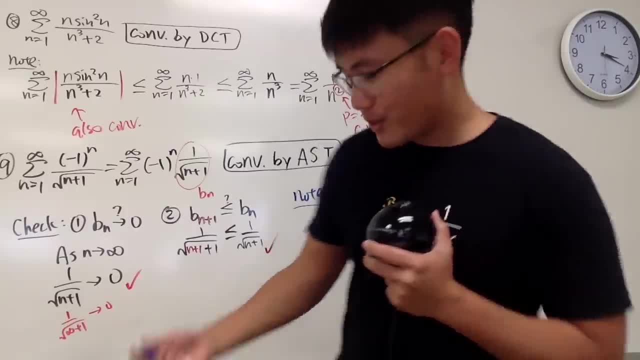 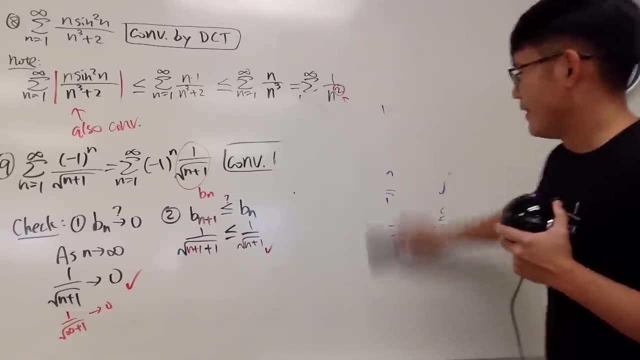 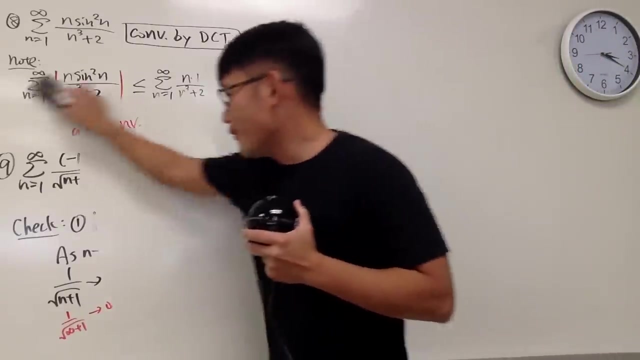 Okay, so hopefully you guys are doing good, And now we are continuing with number 10.. So, in case if you guys wonder why I did integral 100 times and all that, Well, first of all, I'm not going to lie. First of all, it's just because 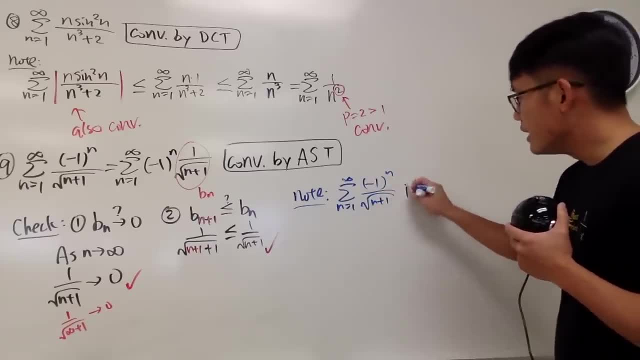 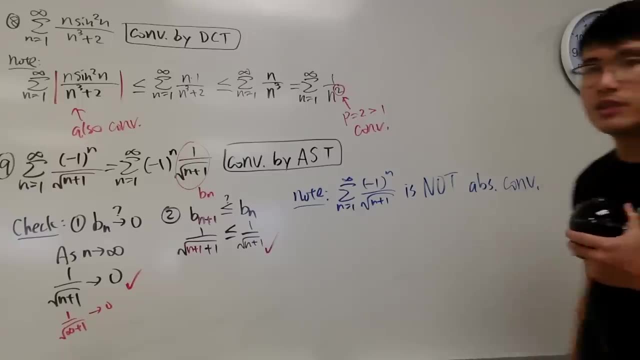 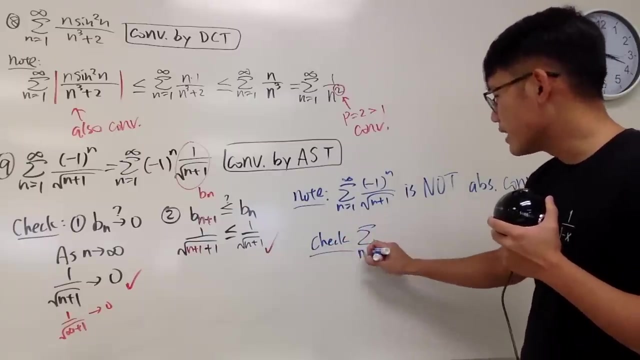 square root of n plus 1.. This, right here, is not absolutely, it's not absolute convergent. It does not converge absolutely Why? Because if you check the limit- sorry, not limit- the sum as n goes from 1 to infinity. if you take the absolute, 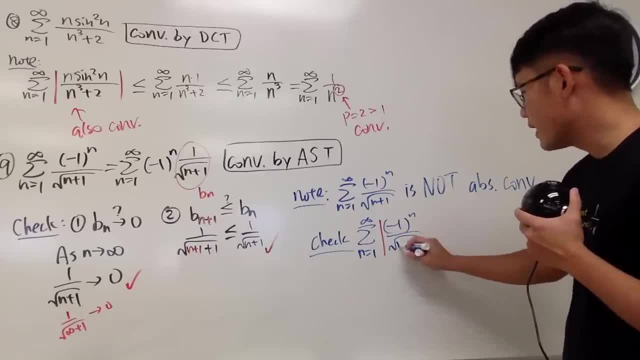 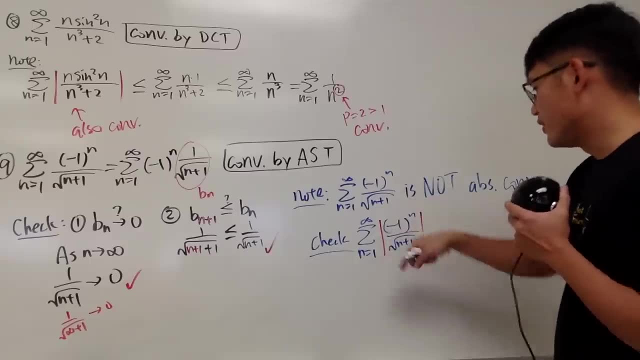 value of this. negative 1 to the nth power over square root of n plus 1, like this: Well, this right here is just 1.. Negative 1 to whatever power: if you have the absolute value, everybody becomes 1.. So this is just n goes. 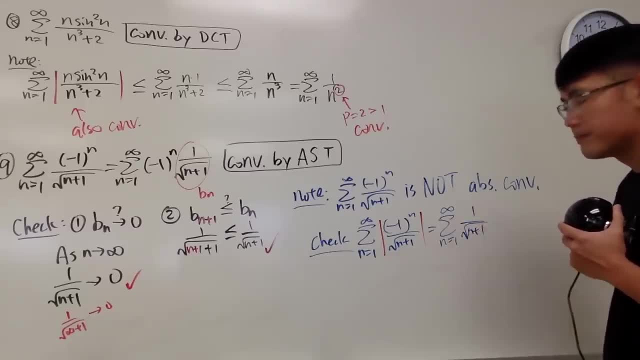 from 1 to infinity of 1 over square root of n plus 1.. And you see the absolute value version of this. you have pretty much an n to the 1 half power if you ignore that and you can do some. 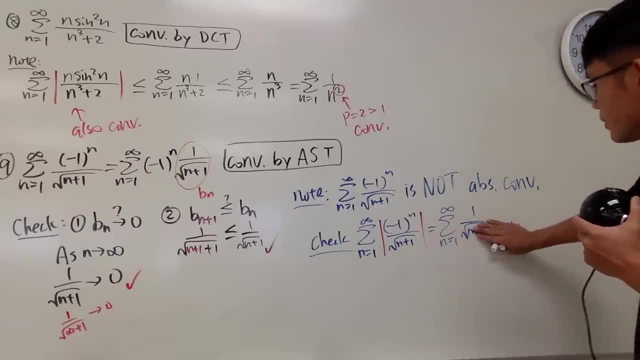 limit compression test if you would like. Right, So you know you can just do the things. yeah, This right here diverges. You can do it by limit compression test with the sum as n goes from 1 to infinity of the square root. 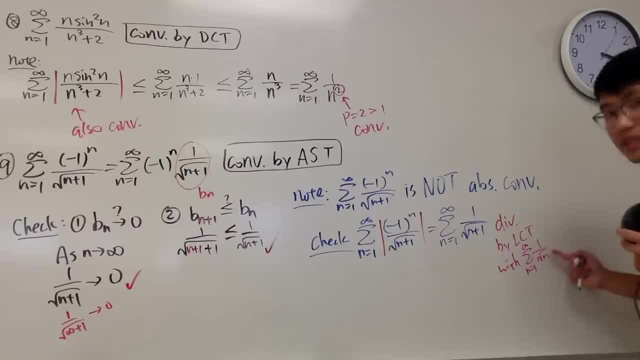 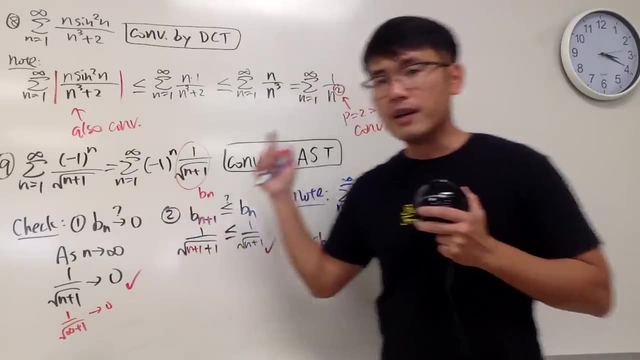 of n like this, Because here the p is 1 half, which is less than 1, less than or equal to 1.. So it diverges. So this right here will be an example of a series that is a convergent but it's not. 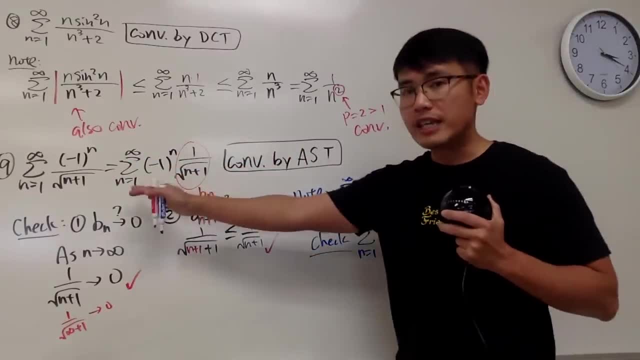 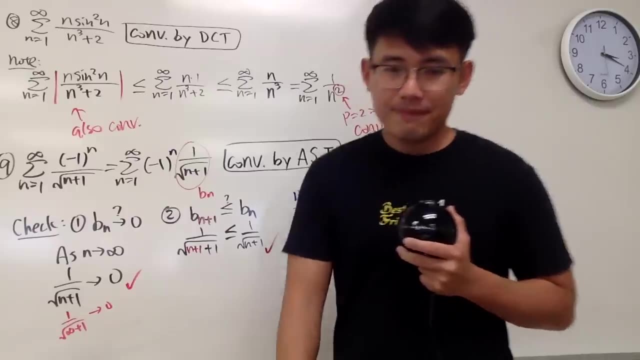 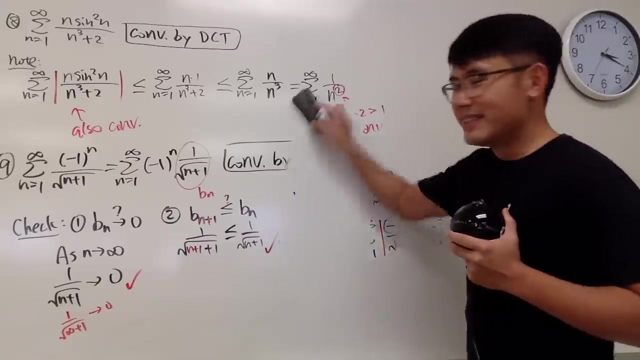 an absolute convergent, And in this case we say this: right, here is a conditional convergent series. right, That's number 9.. Okay, so hopefully you guys are doing good, and now we are continuing with number 10.. 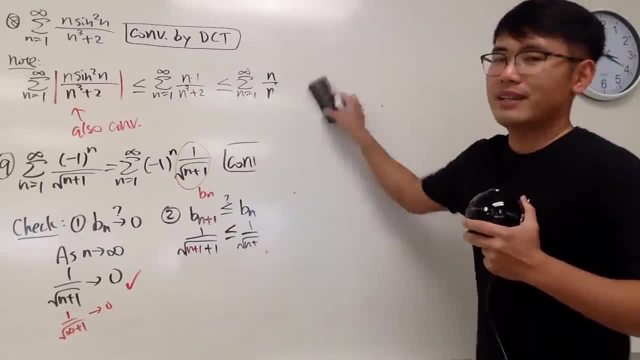 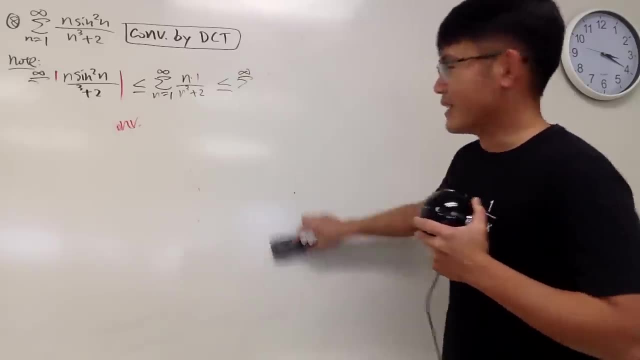 So in case, if you guys wonder why I did integral 100 times and all that, well, first of all, I'm not going to lie. First of all, it's just because the comment Bruce Lee's comment. you guys should know what I'm talking about If you don't. 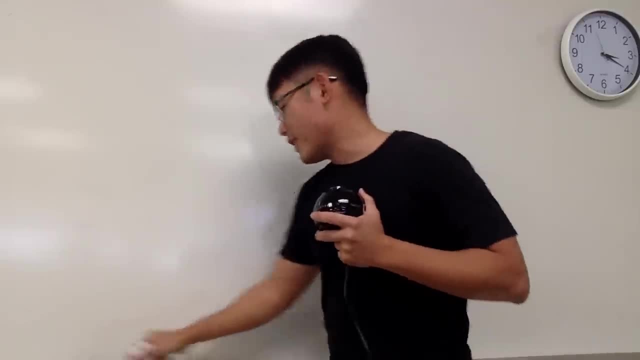 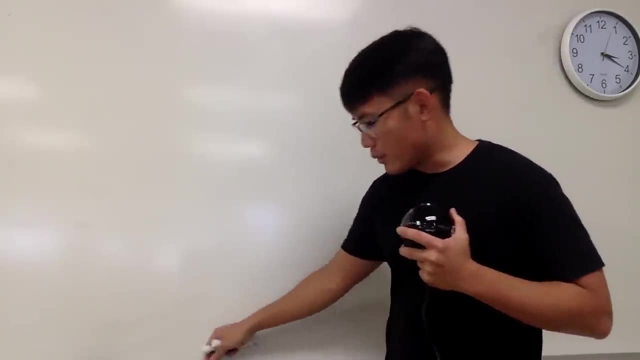 you have to watch more of my videos in order to get my jokes. But second of all, it's a good idea to actually just have just for me to practice. It's just that when I train marathons, I spend about 2-3 hours to run on the street. 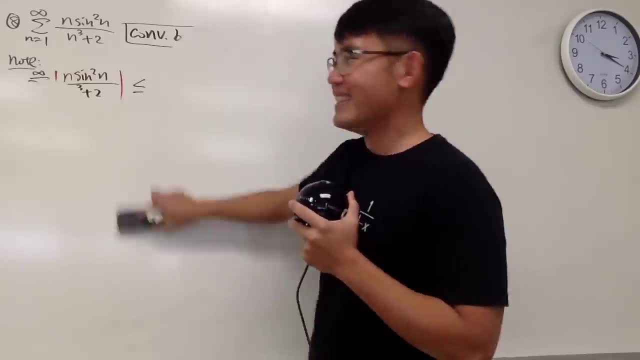 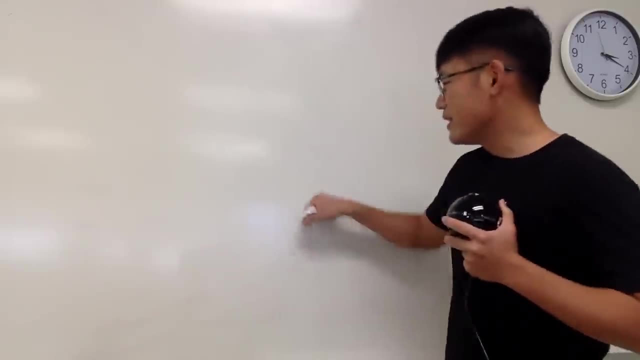 the comment, Bruce Lee's comment. you guys should know what I'm talking about. If you don't, you have to watch more of my videos in order to get my jokes. But second of all, it's a good idea to actually just have just 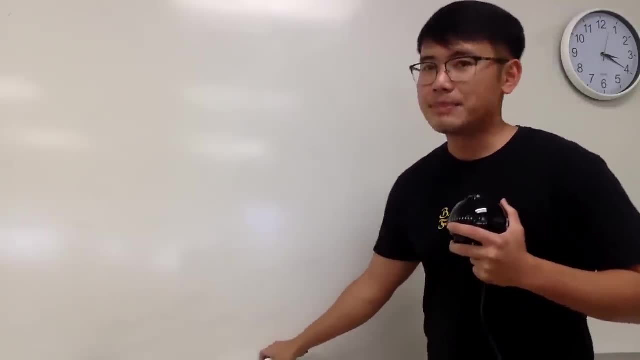 for me to practice. It's just that when I train marathons, I spend about 2-3 hours to run on the street, and then the actual marathons take me like 4-5 hours or so 5 hours. 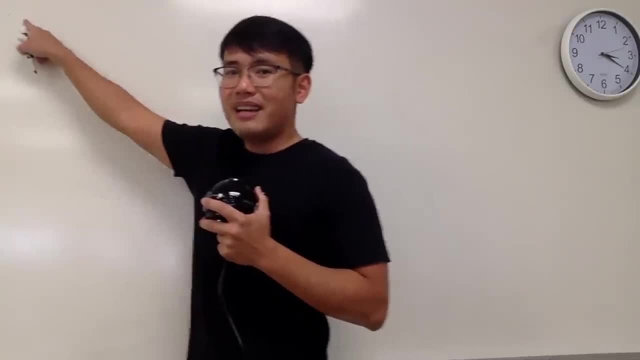 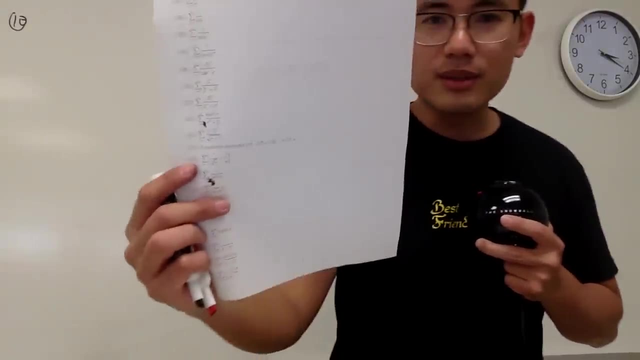 to be honest, because I'm getting old. Anyway, number 10.. If possible, and, by the way, for every question, 10 questions. you guys know the deal: I'll give you guys something special For every 10 questions. 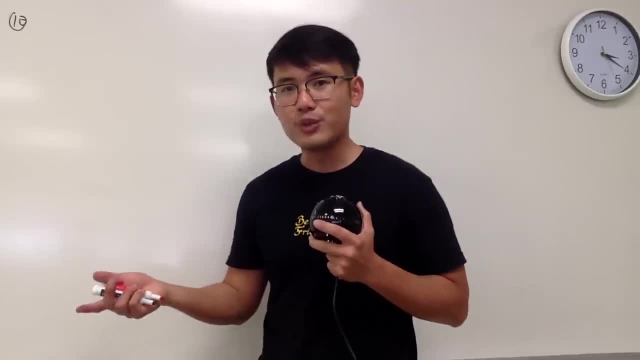 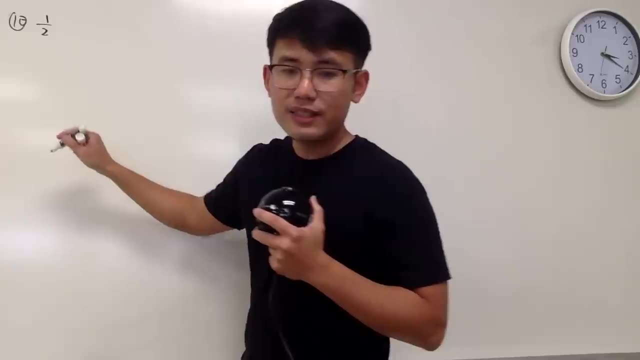 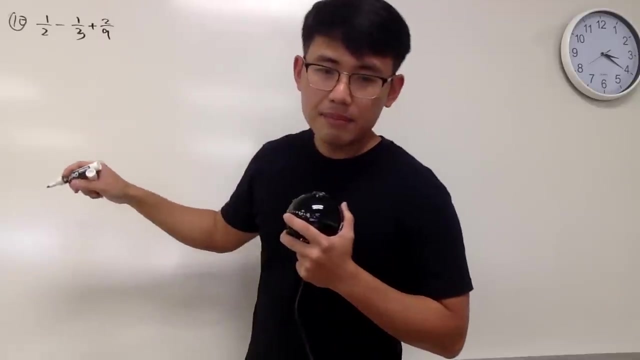 I will be computing the actual sum instead of just telling you guys if it converges or not. So stay tuned for that Number 10,. we are going to calculate 1 half minus 1 third plus 2 over 9 and minus. 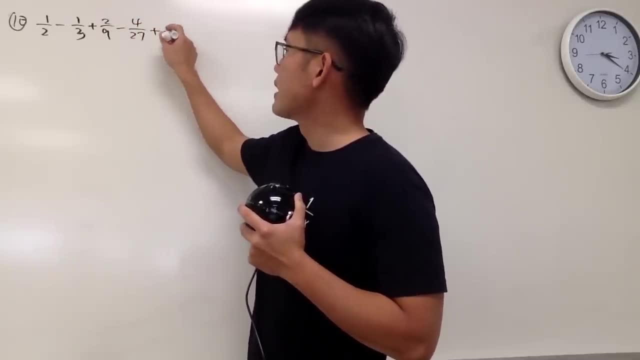 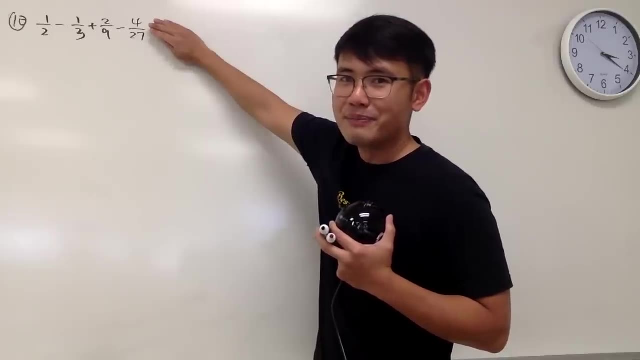 4 over 7.. So 4 over 27. and then, and all that, First of all, if you don't have the plus dot dot dot, this is just basic math. It's crazy because you have lots of fractions Anyway. 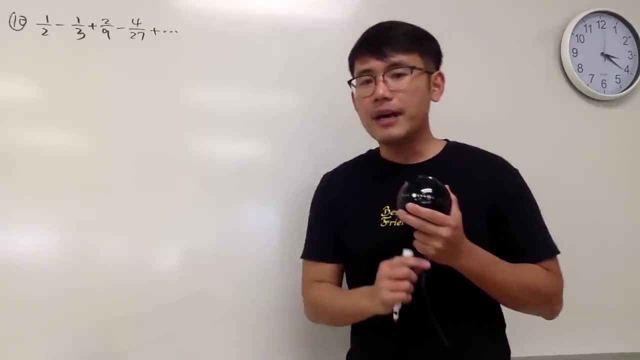 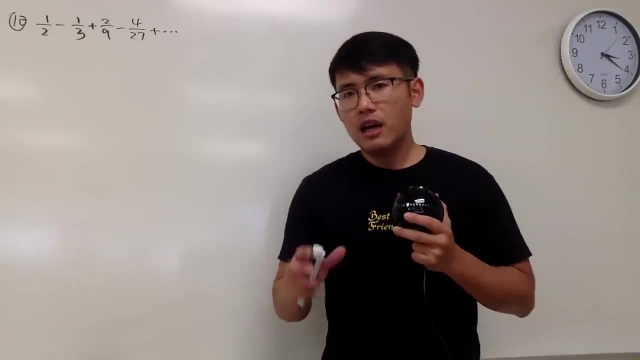 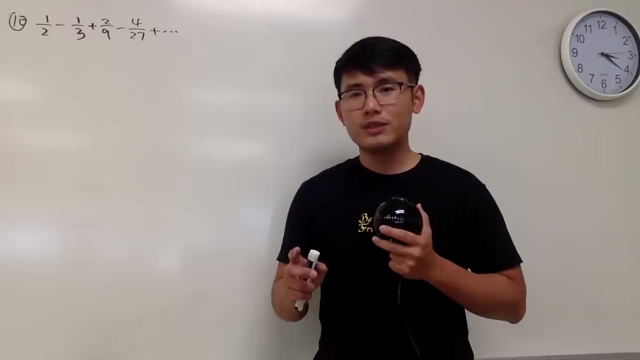 when you have the plus dot dot dot. this is calculus. So that's the cool part. Okay, How can we do this? Well, let me just tell you guys that we can only compute the series in some special situations, And one of the easy ones to compute. 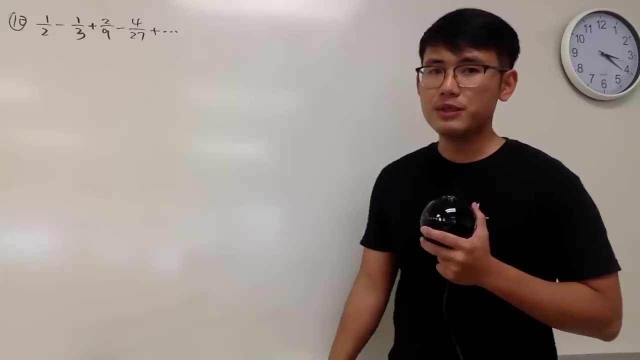 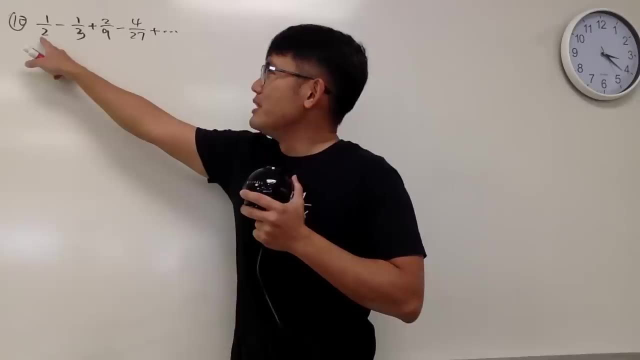 is if this is a geometric series or maybe a telescoping series. The truth is, this is a geometric series. It may not be easy to see from here to here, but from here to here you can see that on the top, we multiply by 2, on the bottom we 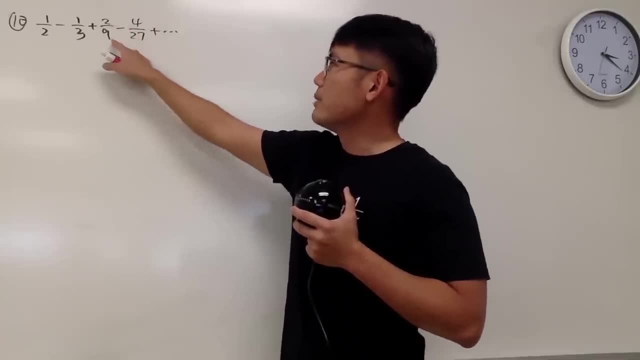 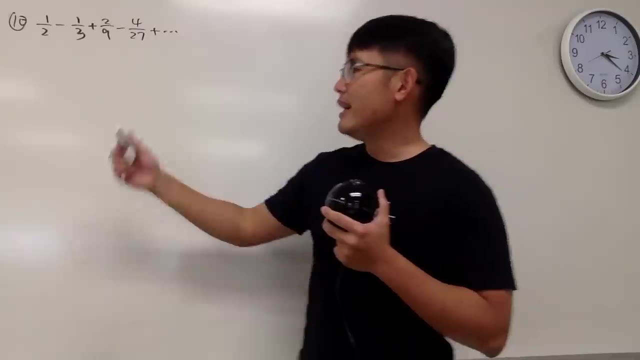 multiply by 3.. On the top, we multiply by 2,, on the bottom, we multiply by 3. And of course the signs alternate. so we have to multiply by a negative r right? So that's the idea And here's the deal. Let me show you guys. 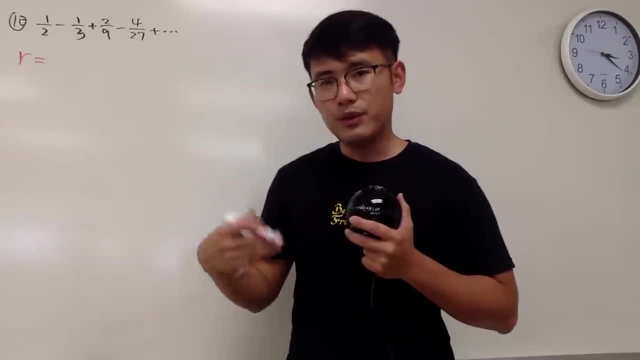 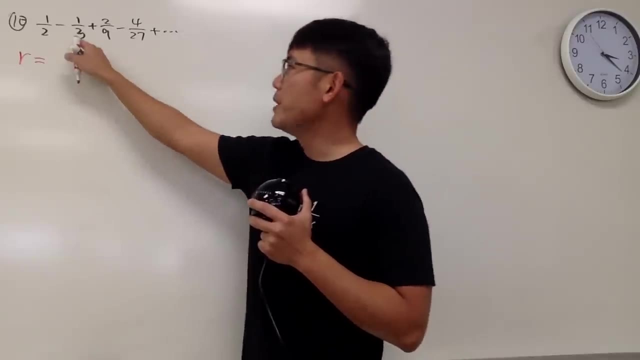 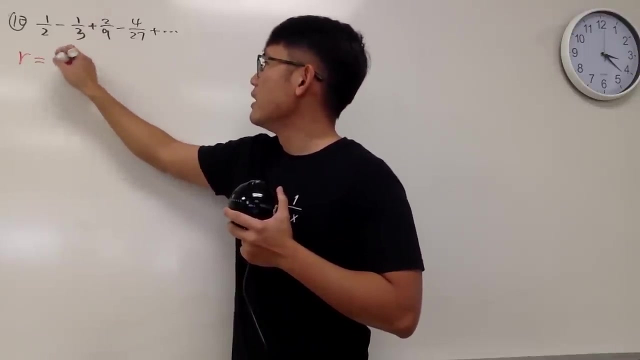 how we can calculate the r in general. if you suspect a series is geometric, First you pick any term, And I'm going to pick this term because these two terms that I don't know what's going on. So I just put negative 1, third, and then 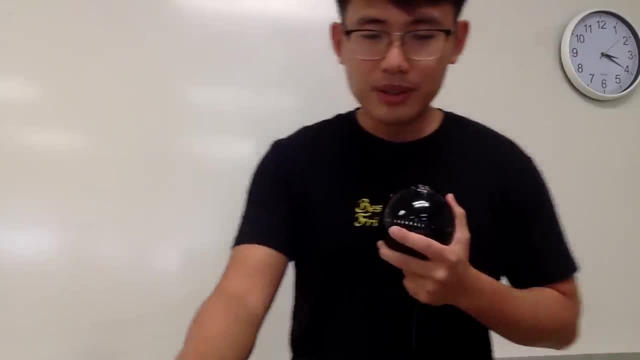 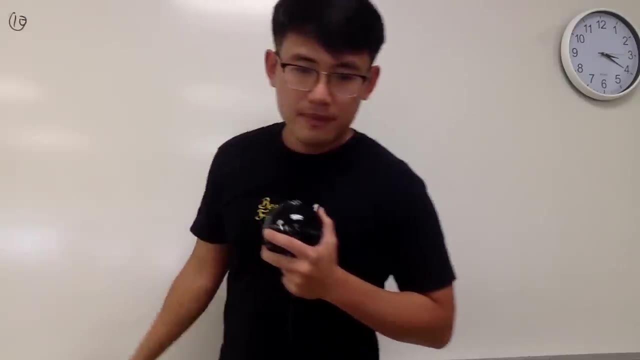 and then the actual marathons. you know take me like 4-5 hours or so- 5 hours, to be honest, because I'm getting old. Anyway, number 10.. If possible, and by the way, for every question, 10 questions. 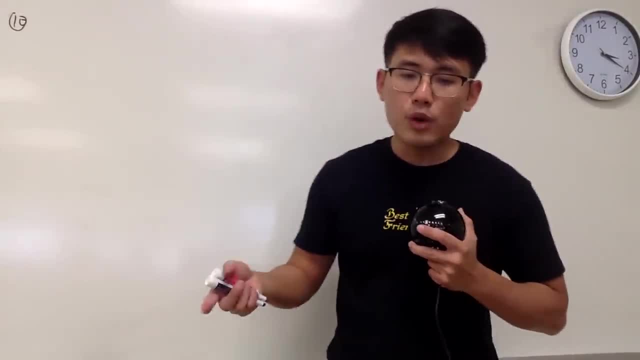 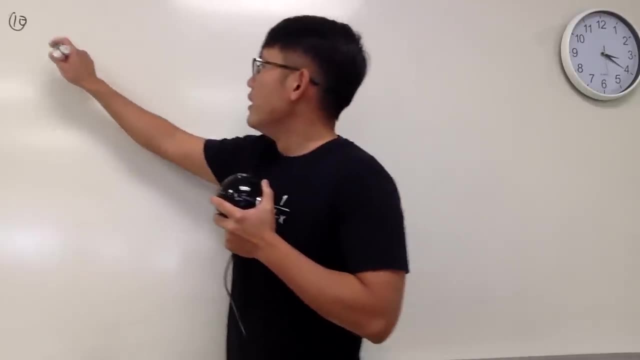 you guys know the deal: I'll give you guys something special: For every 10 questions, I will be computing the actual sum instead of just telling you guys if it converges or not. So stay tuned for that Number 10, we are going to calculate. 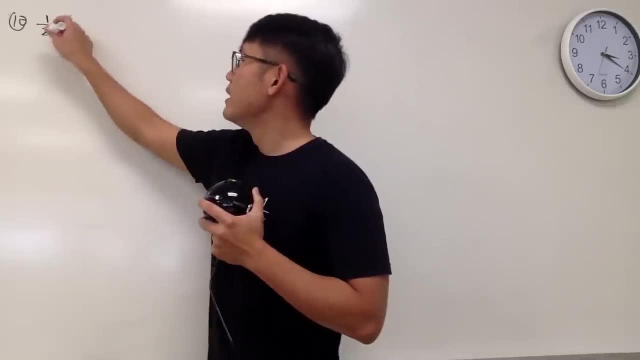 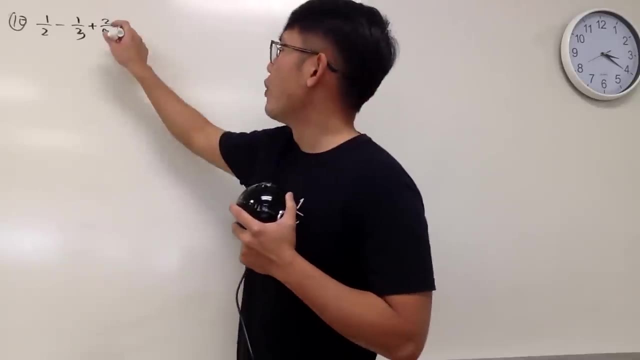 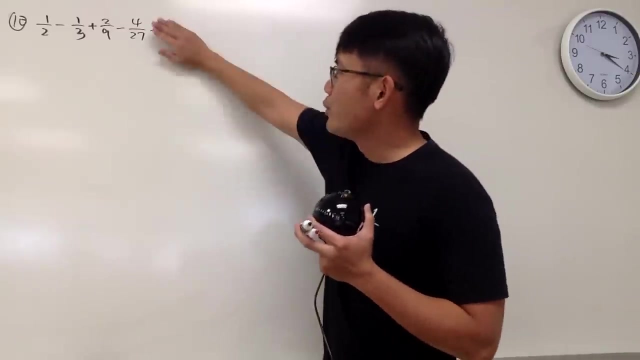 1 half minus 1 third, plus 2 over 9 and minus 4 over 7.. So 4 over 27,, and then dot, dot dot. and all that, First of all, if you don't have the plus, dot, dot dot. this is just basic math. 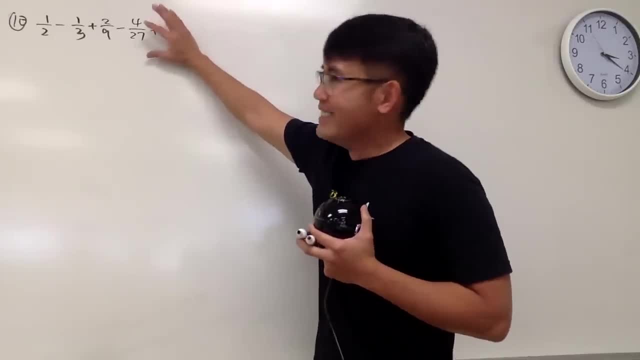 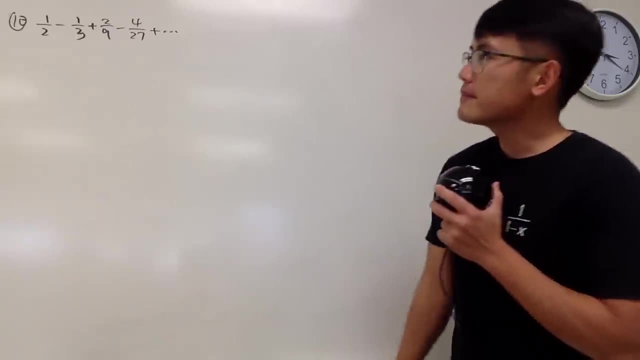 It's crazy because you have lots of fractions. So yeah, Anyway, when you have the plus dot dot dot, this is calculus. so that's the cool part. Okay, How can we do this? Well, let me just tell you guys that. 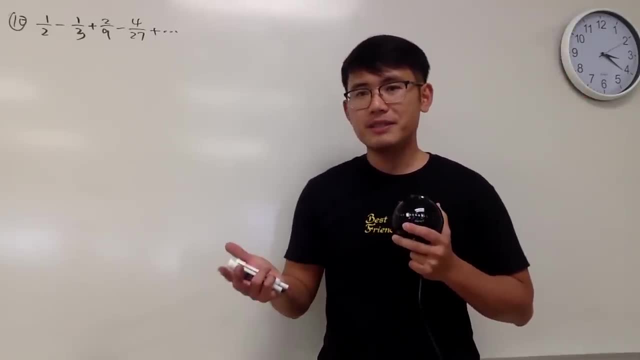 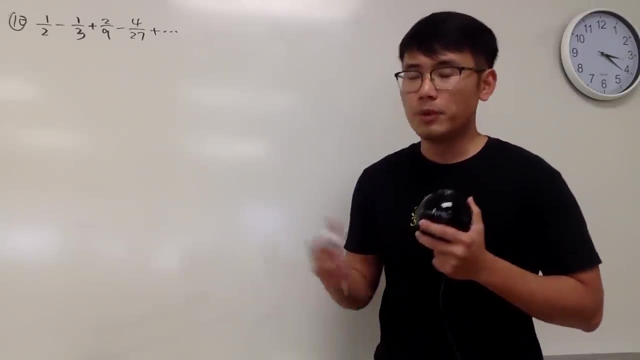 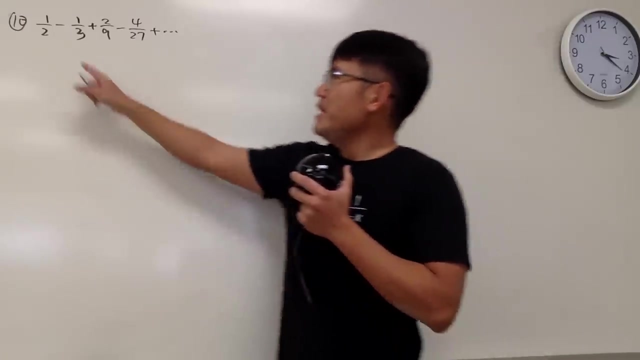 we can only compute the series in some special situations, And one of the easy ones to compute is if this is a geometric series or maybe a telescoping series. The truth is, this is a geometric series. It may not be easy to see from here to here, but 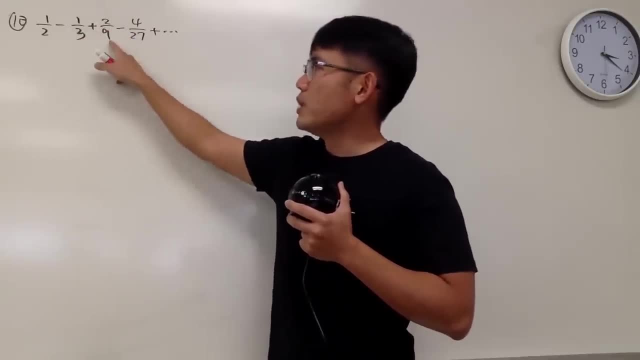 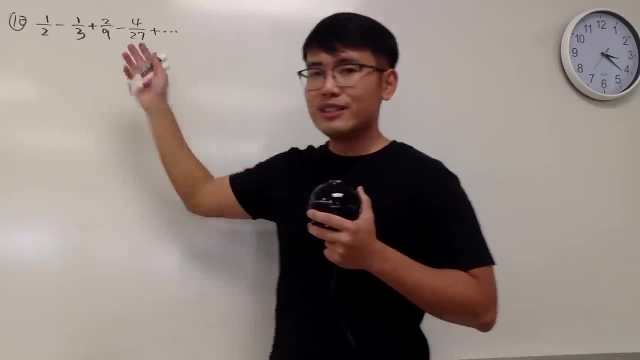 from here to here, you can see that on the top we multiply by 2,, on the bottom we multiply by 3.. And of course the signs alternate, so we have to multiply by a negative r right? So that's the idea. 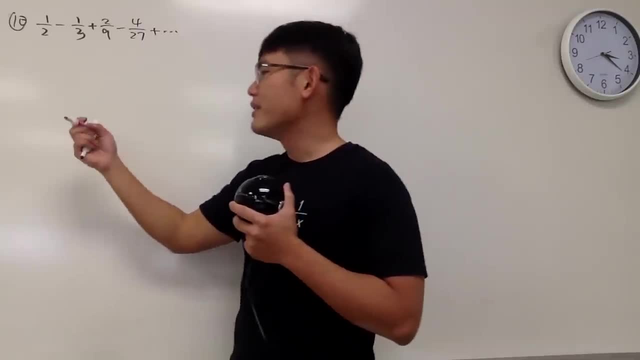 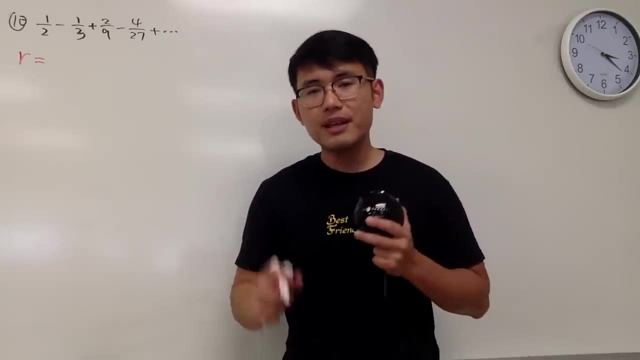 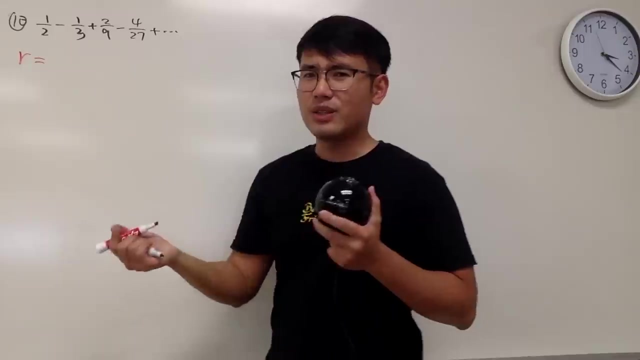 And here's the deal. Let me show you guys how we can calculate the r in general. if you suspect a series is geometric, First you pick any term, And I'm going to pick this term because these two terms, I don't know what's going on. 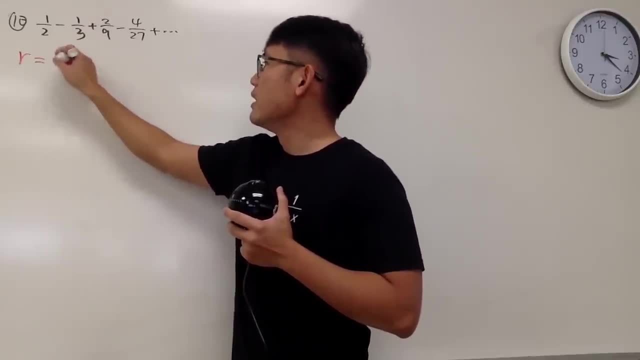 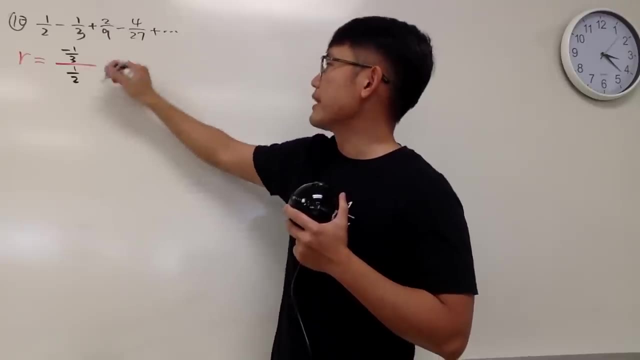 So I just put negative one-third and then I'm going to divide it by its previous term, Which is one-half. Well, you can take the one-half flip like that and you get negative two-thirds. Great. And now notice. 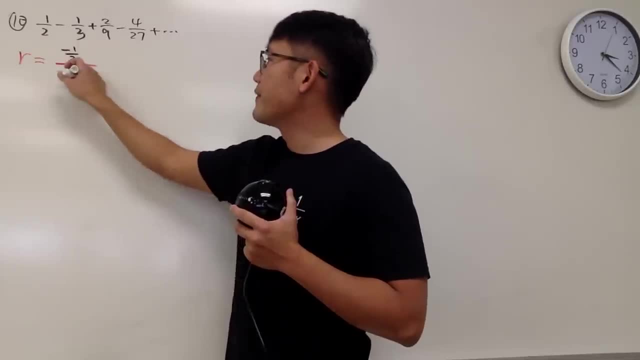 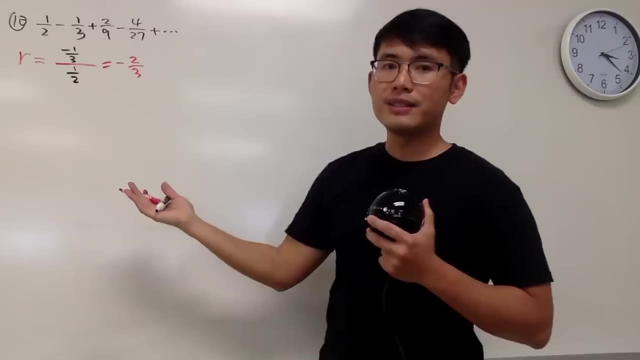 I'm going to divide it by its previous term, which is 1 half. Well, you can take the 1 half, flip it like that and you get negative 2 third, Great. And now notice, if you take the absolute value of 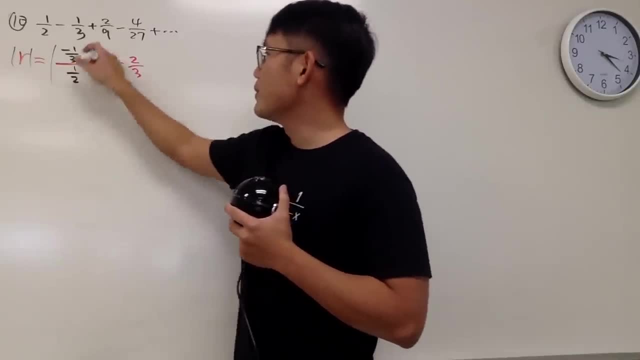 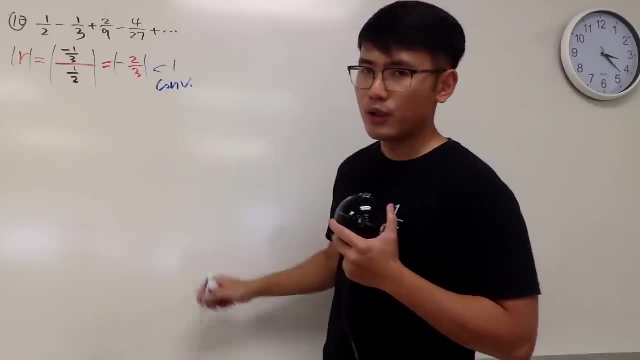 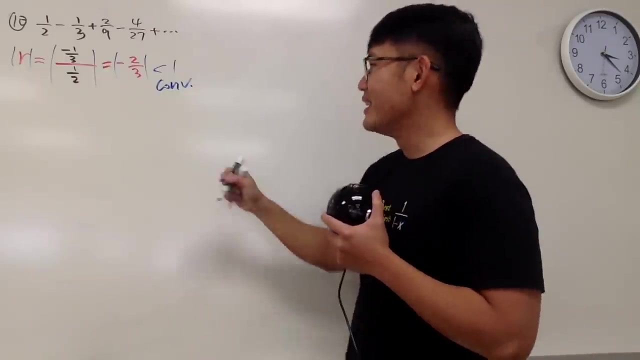 r right here. absolute value of r. absolute value, absolute value: this is less than 1, that means this right here does converge. And now we can use our power of the best friend. We can actually work this out Again. the following only works: 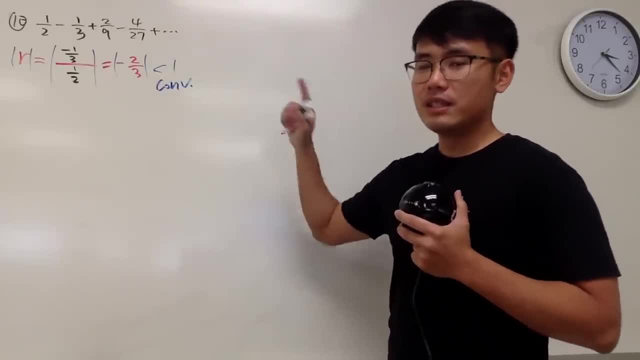 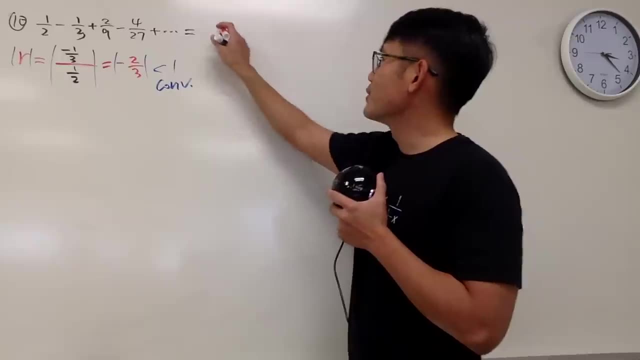 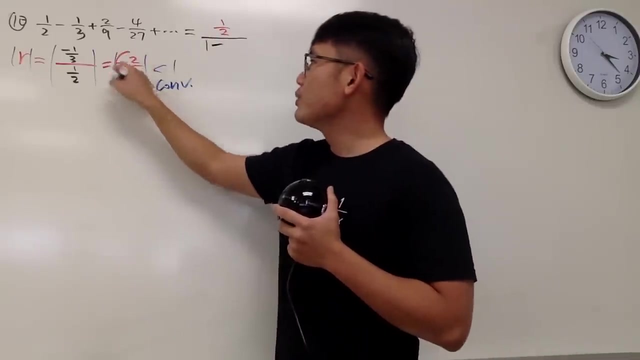 if you have a convergent geometric series- We know this right here will be- you put down the first term, which is 1 half. so I'll just put down 1 half right here, and you divide it by 1 minus the r And you have to use this right. 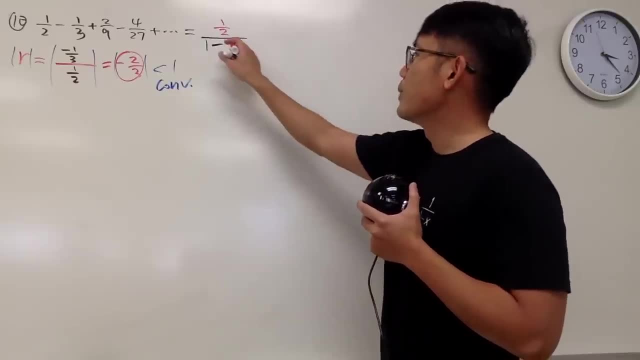 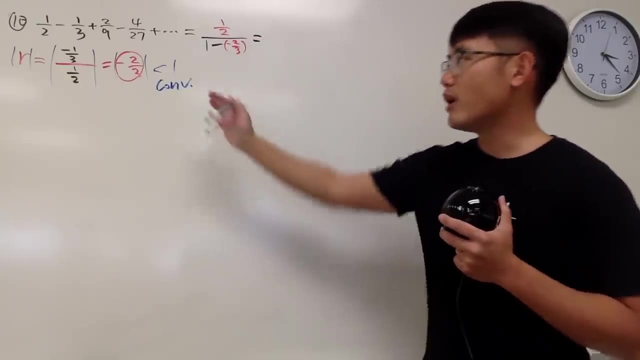 here The r is negative 2 third, So I'll put down negative 2 third like this, And that's it. You have to pay attention to the r, if it converges or not, in order to do this, And the rest is just computing. 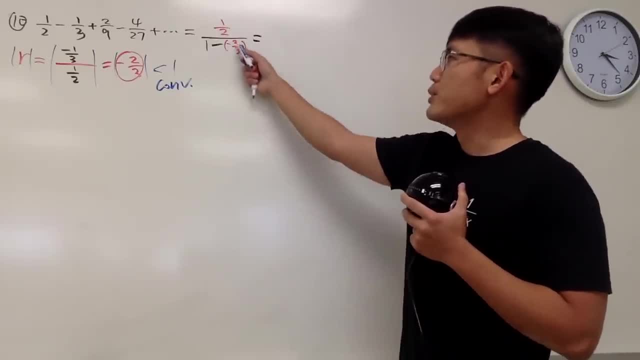 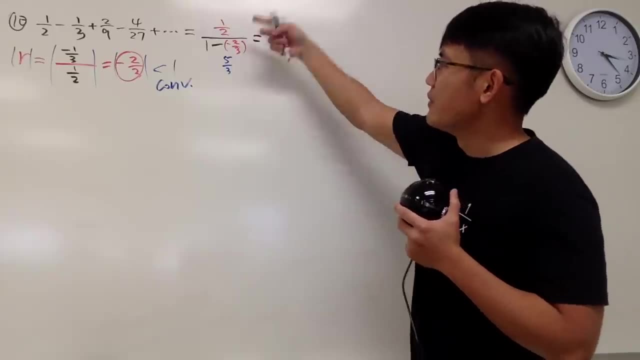 fractions. Okay, let's see 1 plus 2 third. this is as 3 over 3 plus 2 third, which is 5 over 3.. And then you just take this and flip that, so 3 will be on the top. 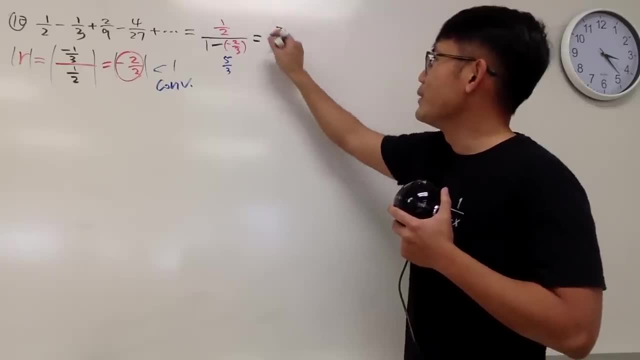 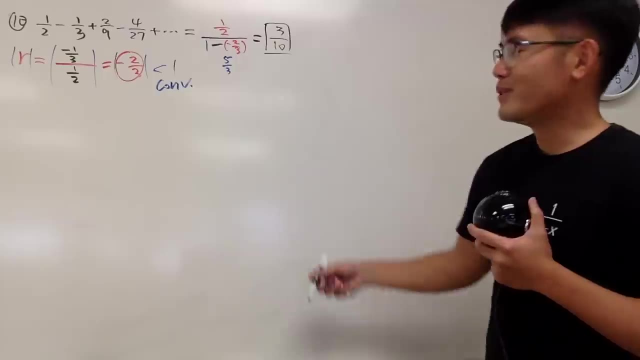 over 2 and 5 will be together and they multiply, which is 10.. So 3 over 10.. And we are all adults now. we are not going to put on decimal, so I'll leave it as 3 over 10.. So that's it Now. 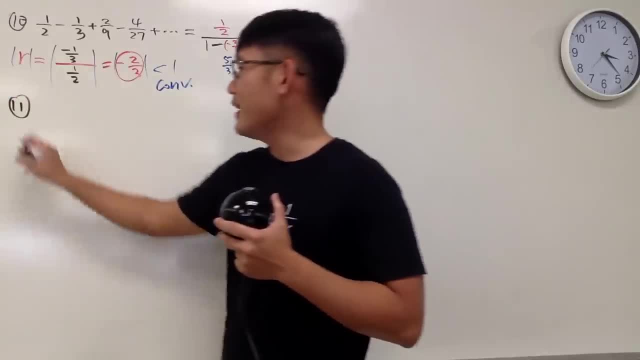 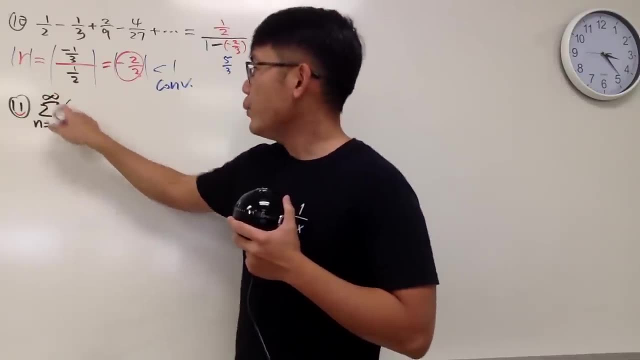 number 11.. It's like a happy face Right here, Number 11.. We are looking at the sum as n goes from 1 to infinity And we have this: 1 over square root of n minus 1 over n. First of all, 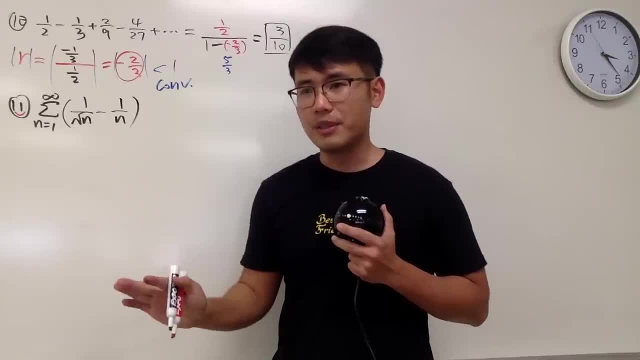 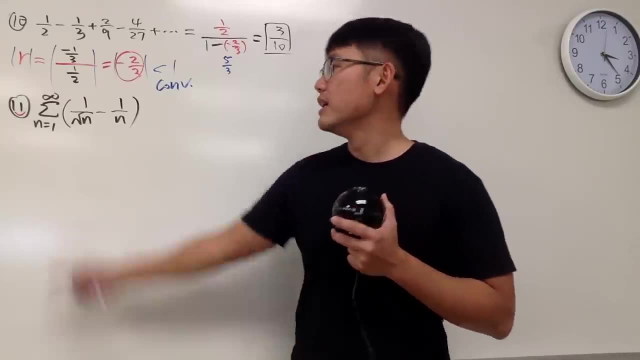 let me give you guys a warning: This, right here, is not a telescoping series. Okay, The people who are watching the YouTube, who are watching the iPhone version, Because this and that they are not of the same kind. Here we have the square root. 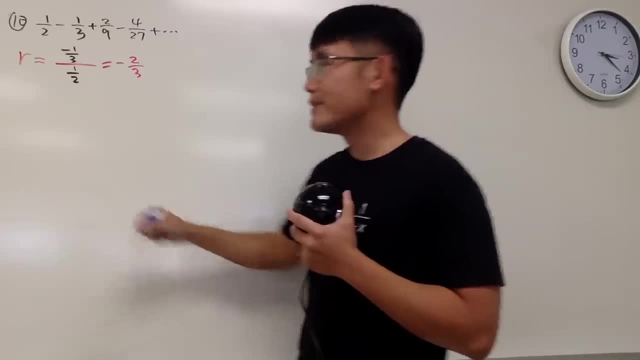 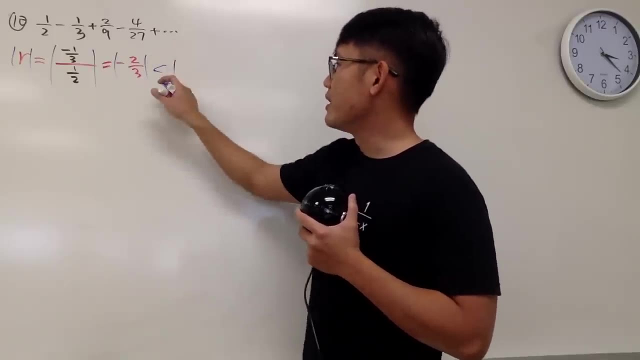 if you take the absolute value of r right here, absolute value of r, absolute value of u, absolute value of u- this is less than 1.. That means this, right here, does converge, And now we can use our power of the best friend. 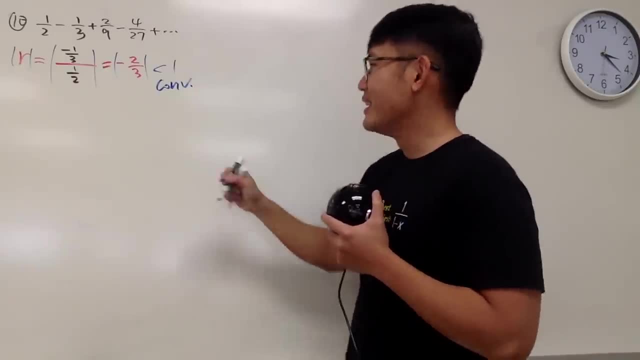 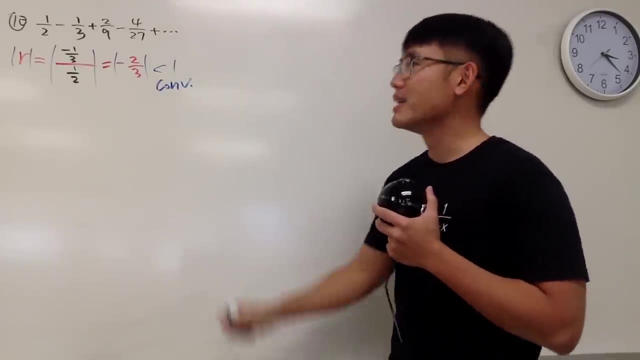 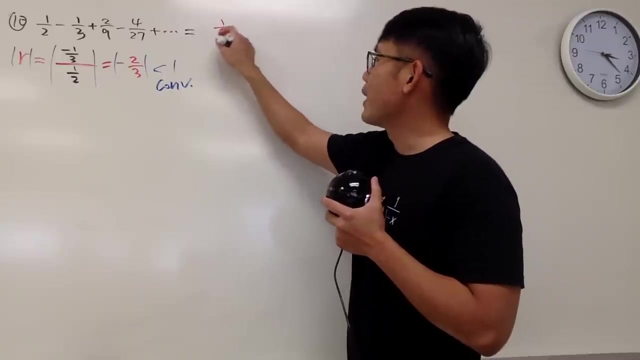 We can actually work this out Again. the following only works if you have a convergent geometric series. We know this. right here will be: you put down the first term, which is one-half. so I'll just put down one-half, right here. 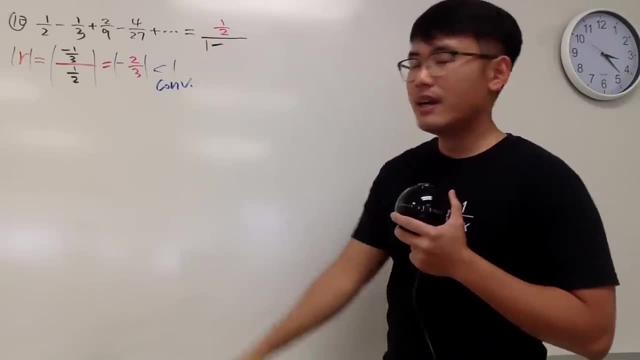 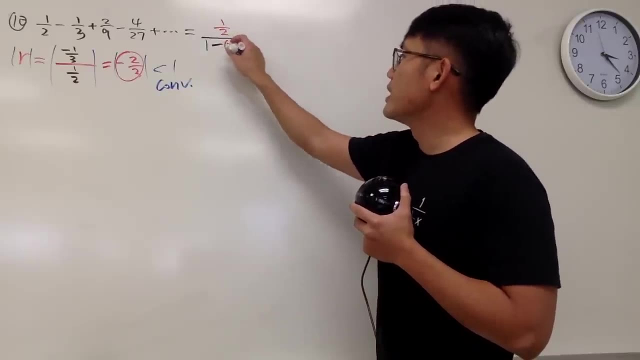 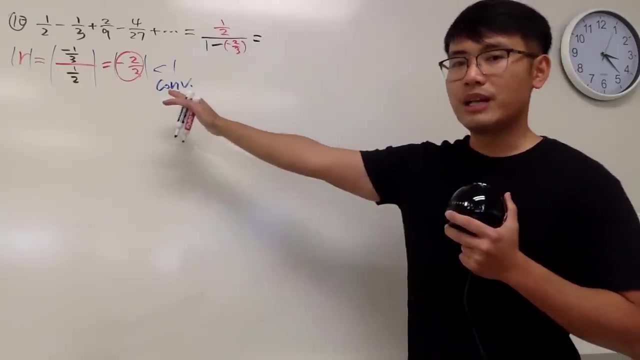 and you divide it by 1 minus the r- And you have to use this right here- The r is negative two-thirds. So I'll put down negative two-thirds like this, And that's it. You have to pay attention to the r, if it converges or not, in order to 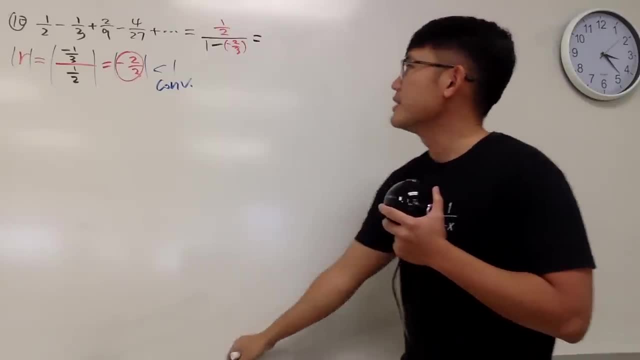 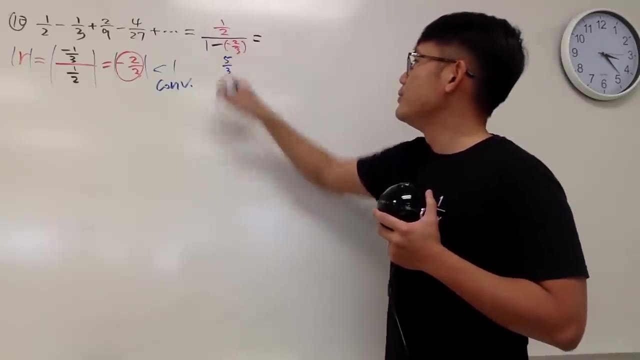 lose this And then the rest is just computing fractions. Okay, let's see 1 plus two-thirds: This is 3 over 3 plus 2-thirds, which is 5 over 3.. And then you just take this and flip that, so 3 will be on the top. 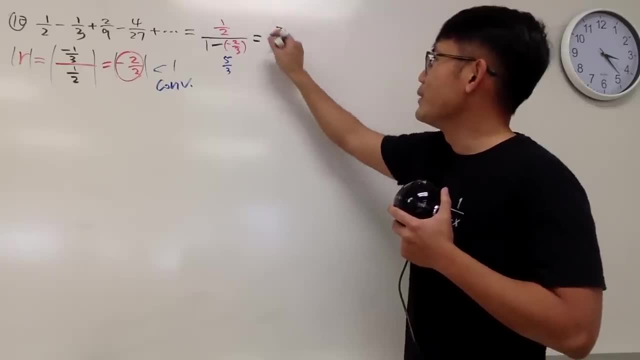 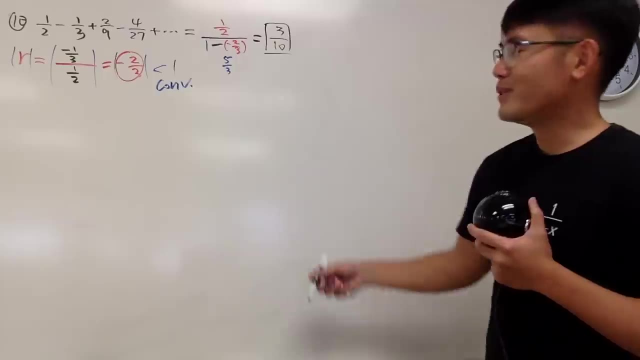 over 2 and 5 will be together and they multiply, which is 10.. So 3 over 10.. And we are all adults now. We are not going to put on decimal, so I'll leave it as 3 over 10.. So that's it Now. 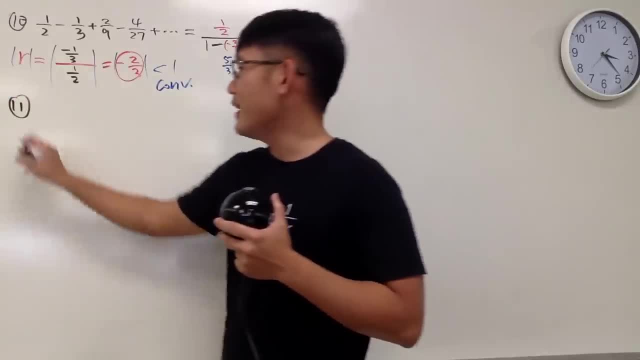 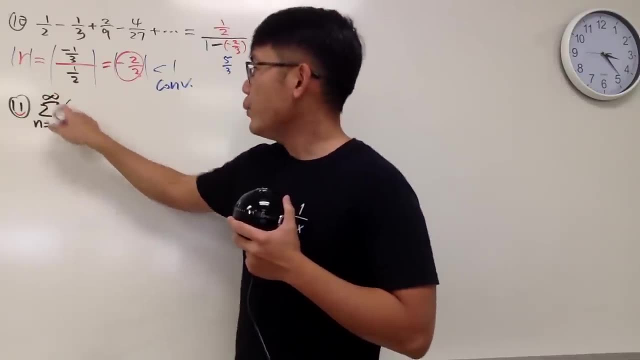 number 11.. It's like a happy face Right here, Number 11.. We are looking at the sum as n goes from 1 to infinity And we have this: 1 over square root of n minus 1 over n. First of all, 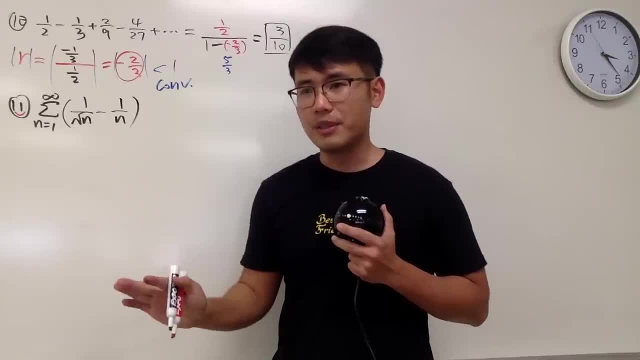 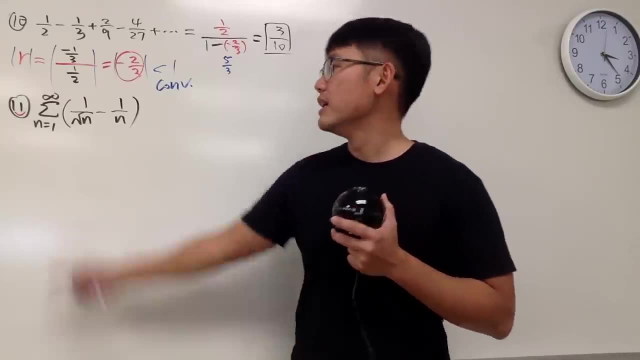 let me give you guys a warning: This, right here, is not a telescoping series. Okay, The people who are watching the YouTube, who are watching the iPhone version, Because this and that they are not of the same kind. Here we have the square root. 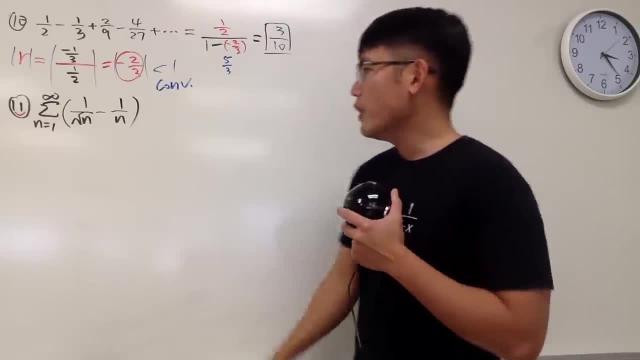 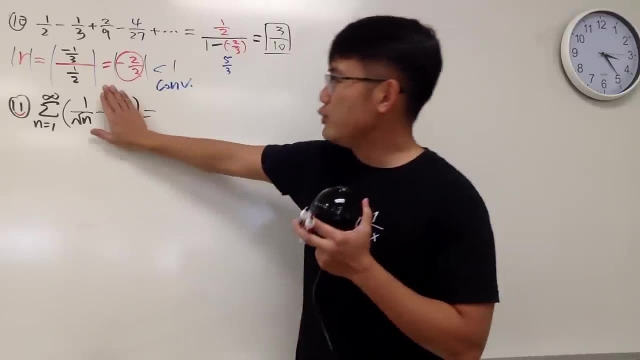 of n. This right here is just n, Totally different things. Well, first of all, of course, we can combine the fractions and do all that, but let me mention this first. If you just have this, the sum of 1 over square root. 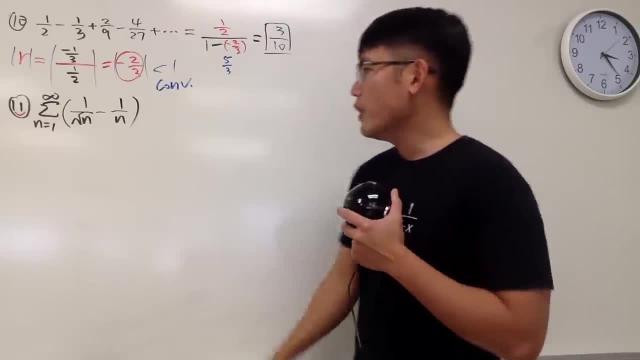 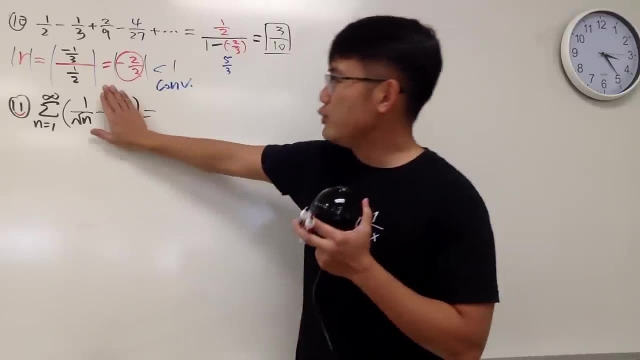 of n. This right here is just n. The total is different things. Well, first of all, of course, we can combine the fractions and do all that. but let me mention this first: If you just have this, the sum of 1 over square root, 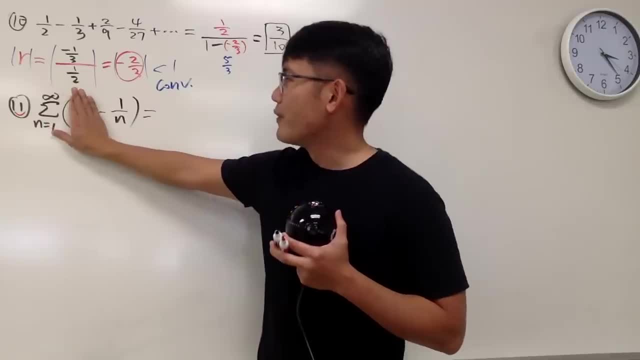 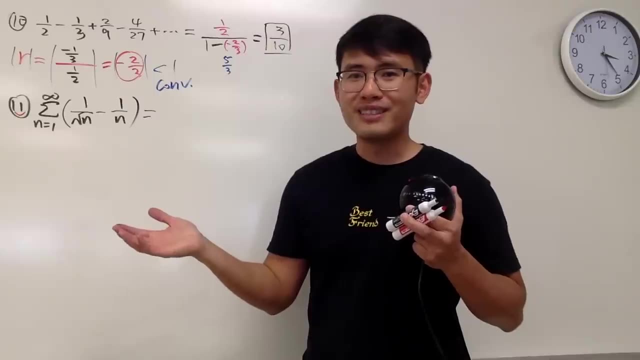 of n. it diverges The sum of 1 over n. it also diverges When you have a divergent minus a divergent. in fact, you don't know what will happen. It may converge, It may diverge. 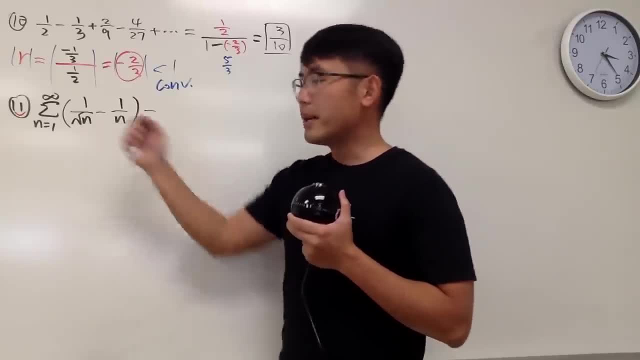 That's the deal, right. So let's take a look. I'm going to combine the fractions, Get the common denominator and all that. So here we have the sum, as n goes from 1 to infinity, And the common denominator. 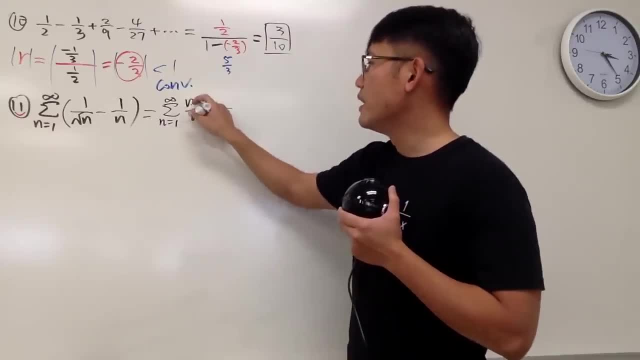 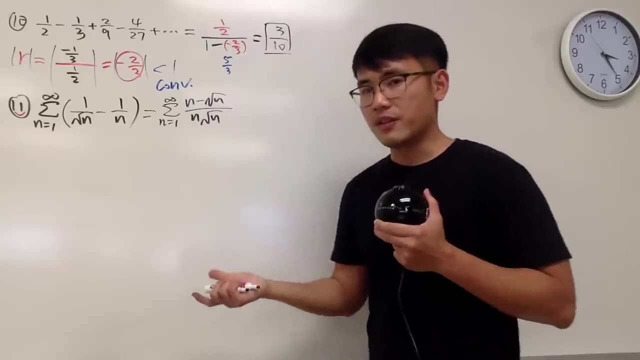 is n, square root of n, And you put the n right there And then you have this right here, And it's always a good idea, I would say, to put things together in a set of fractions, unless it's a telescoping series. 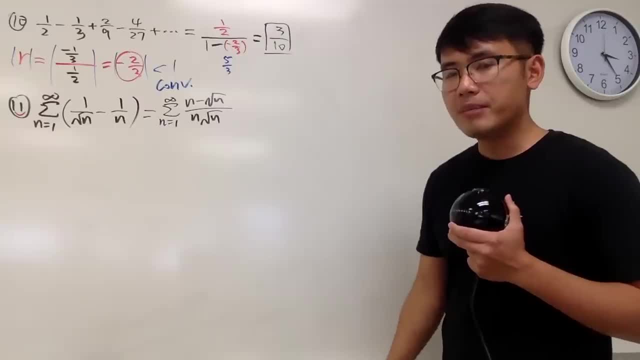 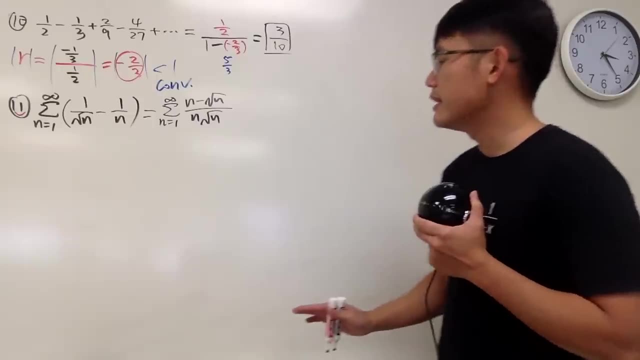 So that's what we have. And now again, let's look at the dominating part, And I think this time we will do a limit comparison test, Not a direct comparison test. Right, Not a direct comparison test, Because if you just 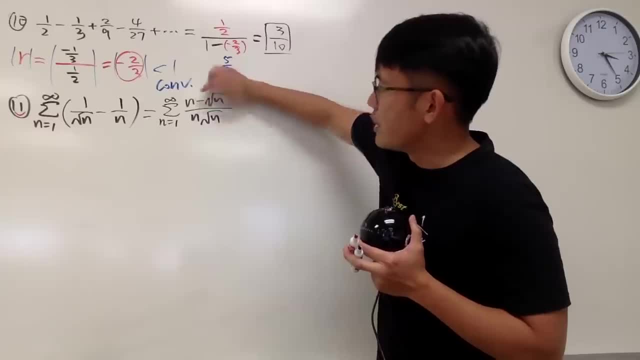 look at the dominating part, you'll see that on the top, we care about this more than that. On the bottom, it's just this. So all in all, we have 1 over square root of n, And that diverges. 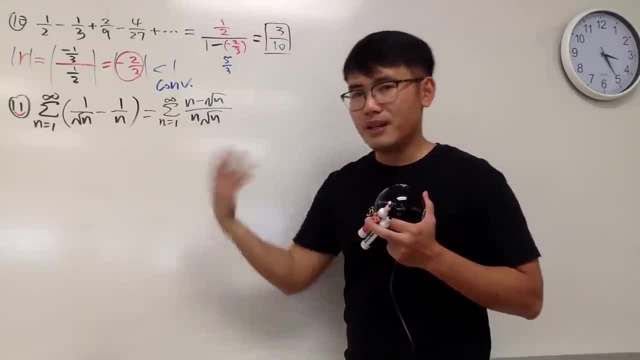 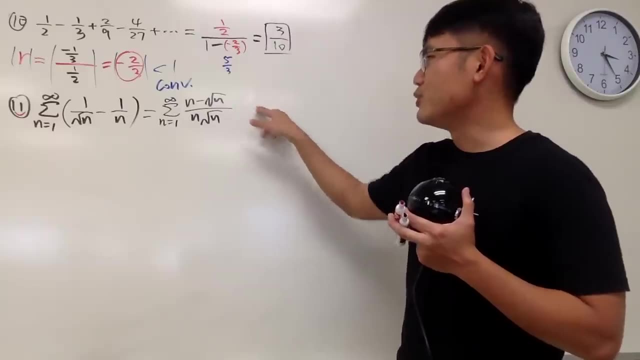 So we are looking for to show. Well, if you want to use a direct comparison test, this is not going to be easy to show. this is greater than or equal to 1 over square root of n. You cannot show this is greater than or equal to. 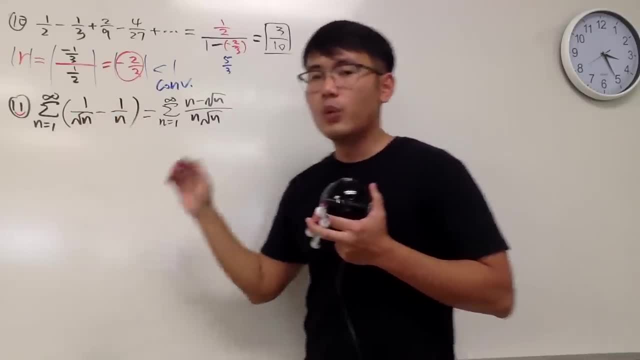 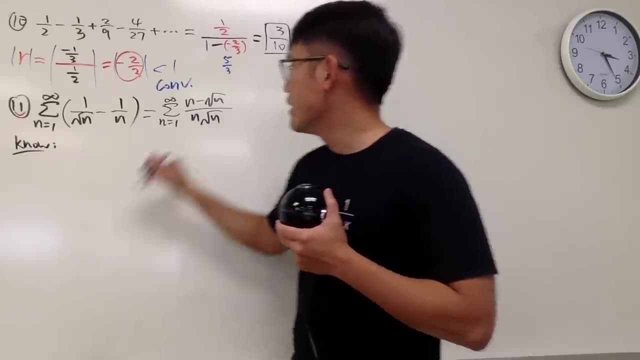 1 over square root of n, Because in fact this is slightly less than 1 over square root of n. Anyway, let me put down what we know Again: pick this and pick that, So we get the sum as n goes from 1. 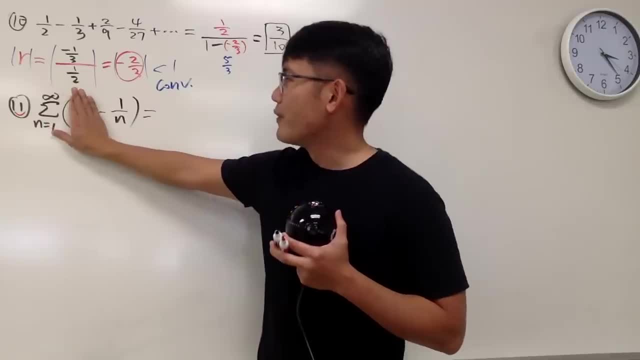 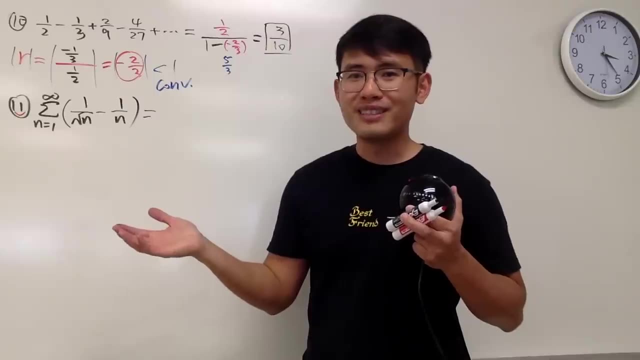 of n. it diverges The sum of 1 over n. it also diverges When you have a divergent minus a divergent. in fact, you don't know what will happen. It may converge, It may diverge. 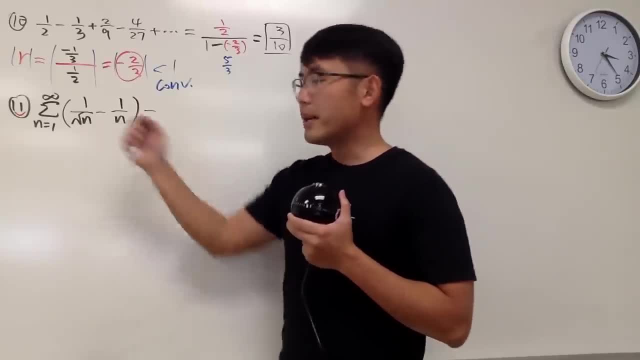 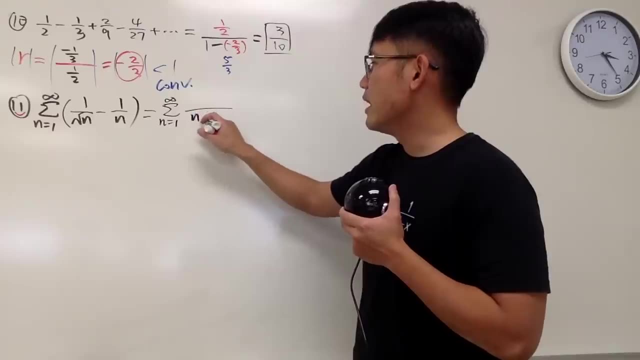 That's the deal, right. So let's take a look. I'm going to combine the fractions, Get the common denominator and all that. So here we have the sum as n goes from 1 to infinity, And the common denominator is n, square root of n. 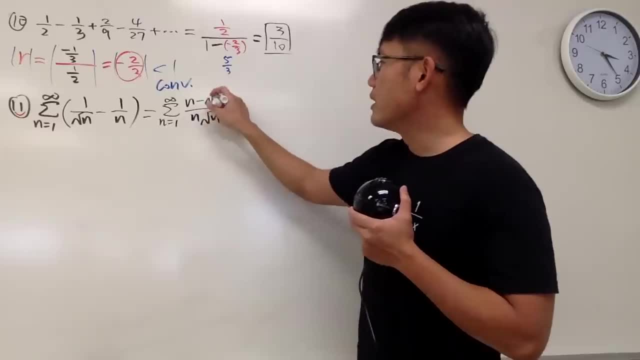 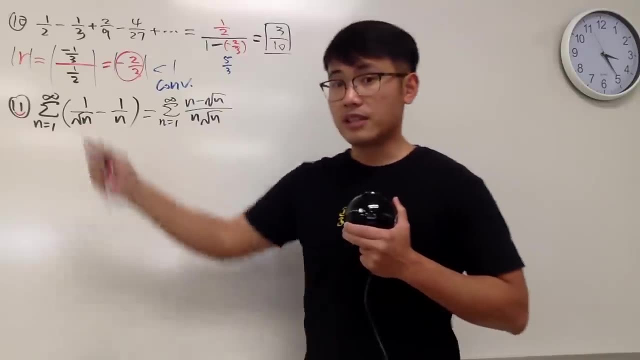 And you put the n right there, and then you have this right here, And it's always a good idea, I would say, to put things together in a set fraction, unless it's a telescoping series. So that's what we have. And now, 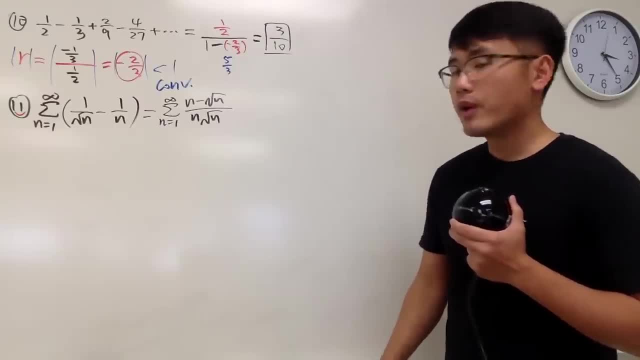 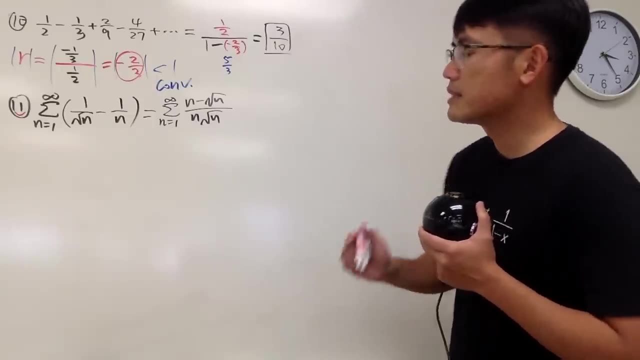 again, let's look at the dominating part, And I think this time we will do a limit comparison test, Not a direct comparison test. Right, Not a direct comparison test? Because if you just look at the dominating part, you'll see that on the top, we care about this. 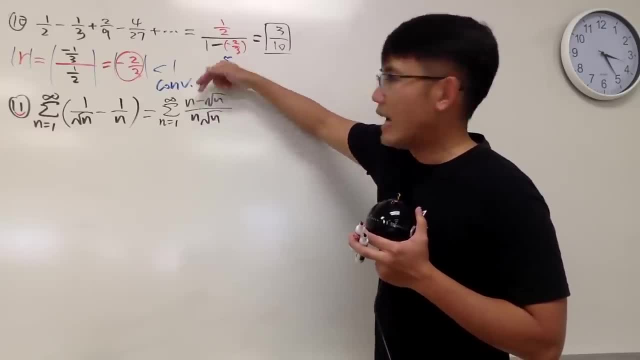 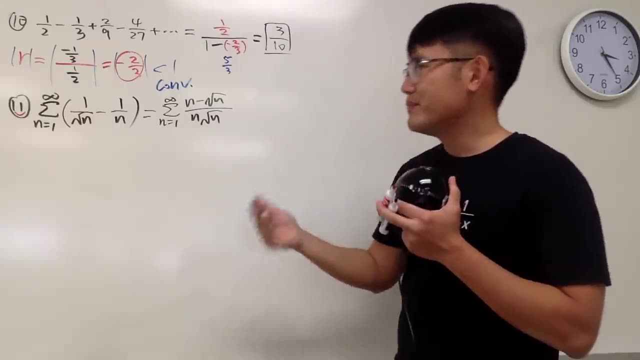 more than that. On the bottom it's just this. So, all in all, we have 1 over square root of n, And that diverges. So we are looking for to show: Well, if you want to use a direct comparison test, this is not going to be. 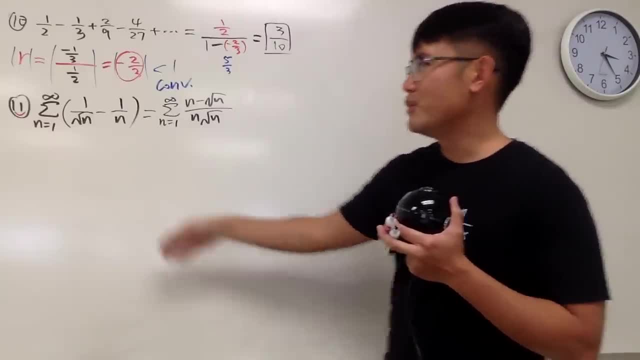 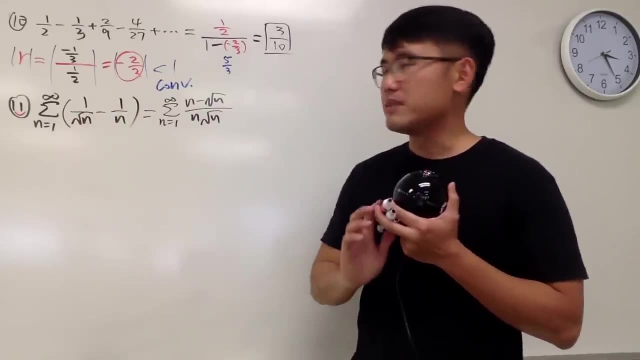 easy to show this is greater than or equal to 1 over square root of n. You cannot show this is greater than or equal to 1 over square root of n, Because in fact this is slightly less than 1 over square root of n. Anyway. 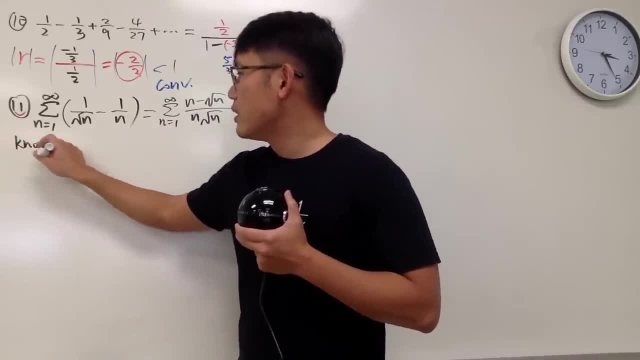 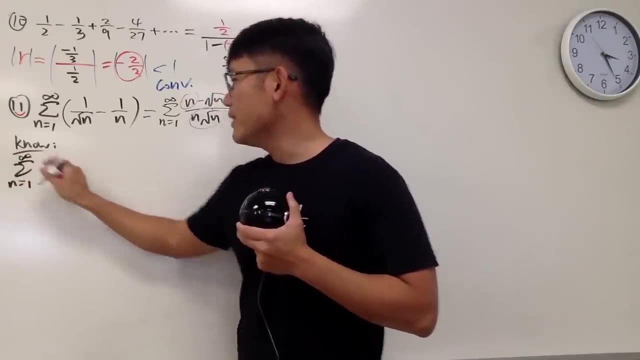 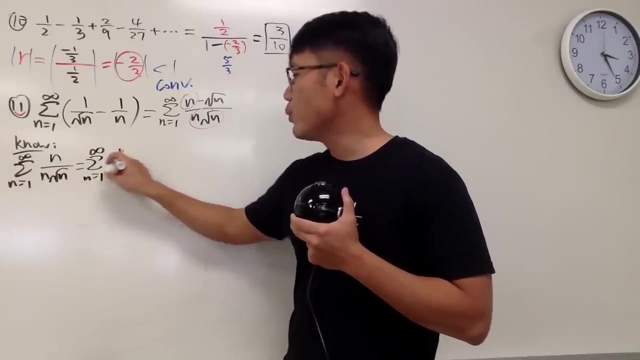 let me put down what we know Again. pick this and pick that, So we get the sum as n goes from 1 to infinity and just n over n square root of n. In other words, the sum as n goes from 1 to infinity. 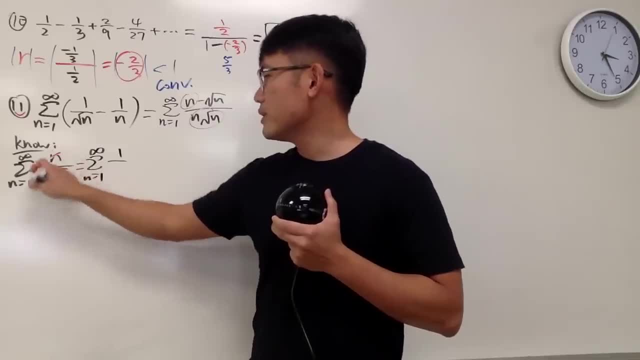 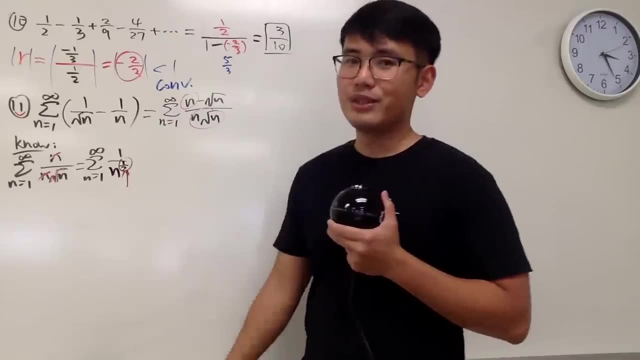 1 over square root of n. only right, Because of course they cancel out And of course this is n to the 1 half power. And now let's do this to be cute. p is 1 half, But you have to mention: 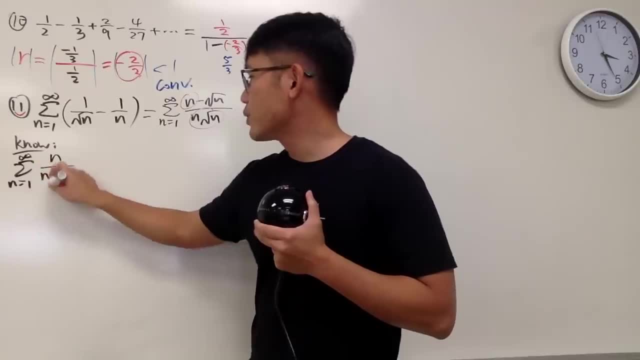 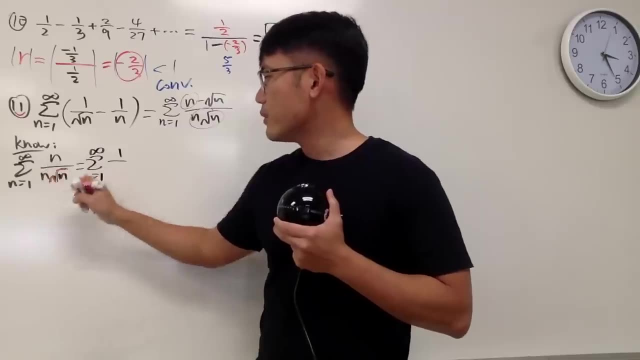 to infinity and just 1 over n, square root of n. In other words, the sum as n goes from 1 to infinity, 1 over square root of n. only Right, Because of course they cancel out And of course this: 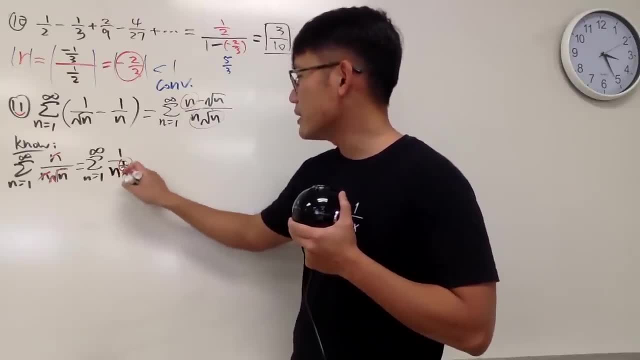 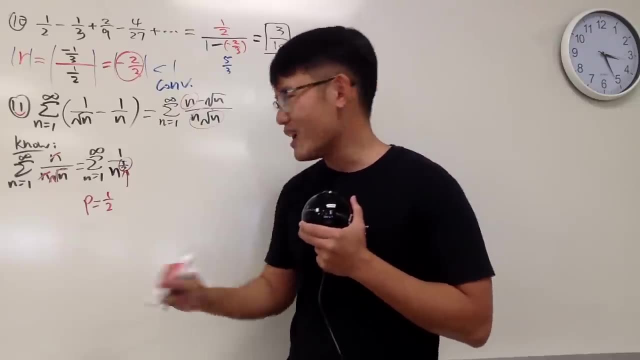 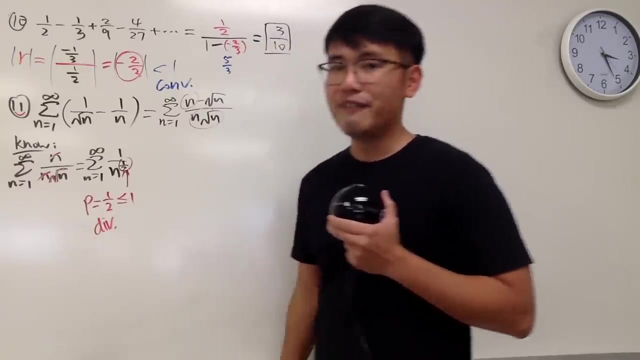 is n to the 1 half power. And now let's do this to be cute: p is 1 half, But you have to mention p is less than or equal to 1.. That's the p series test And this right here diverges. 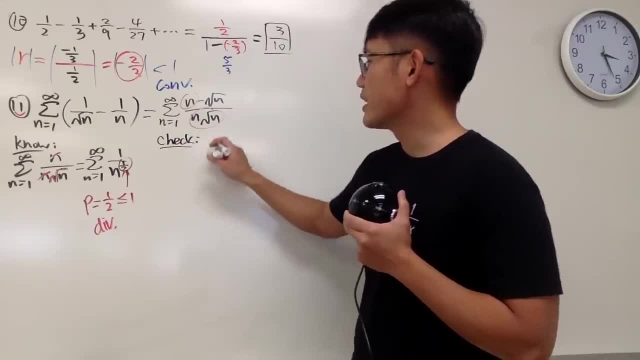 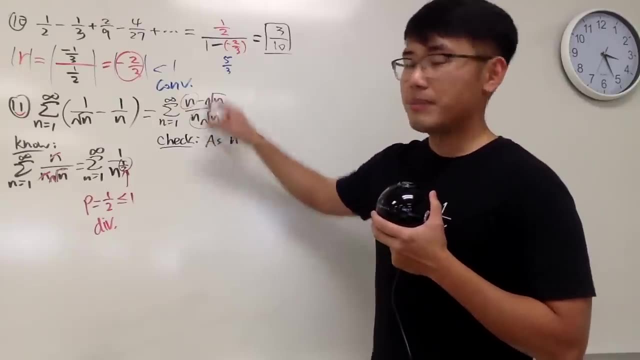 Now we are going to do the check. Well, we take the limit as n goes to infinity, Put down the one that you want to work out on the top right, And the truth is it doesn't really matter. You can put this on the. 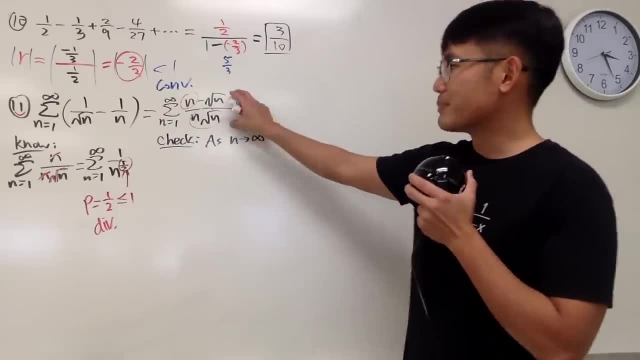 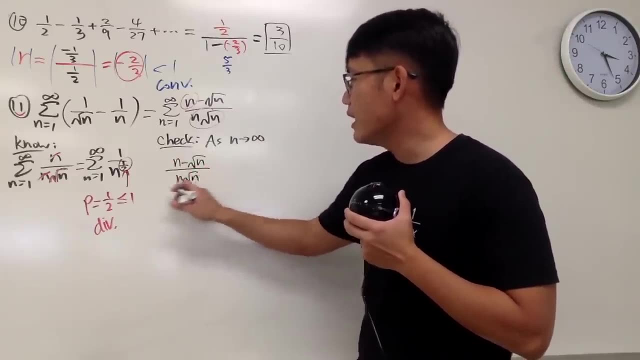 bottom as well. if you like that to be consistent, Let's put this one on the top. So here we have n minus square root of n over n square root of n over. let me just put down over. let me put down one over. 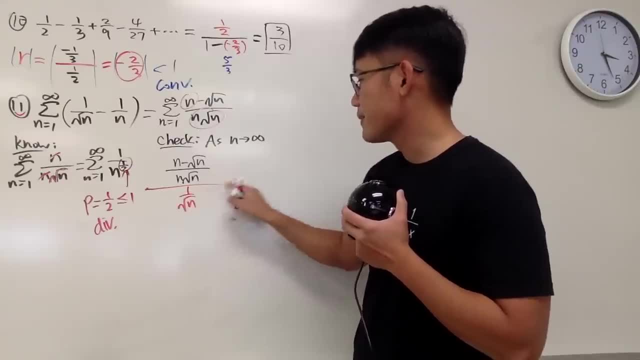 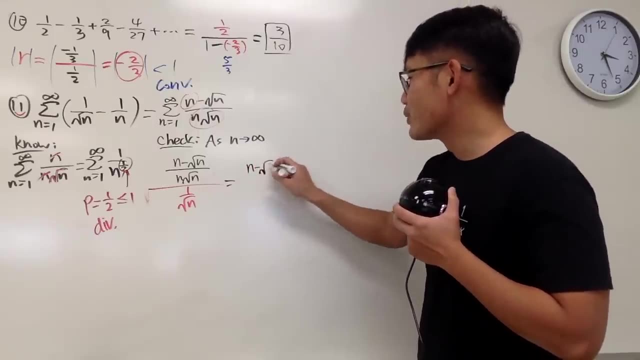 square root of n, because everybody has a square root of n, So why not? So this is what we have Now. do algebra. Take this: so we have n minus square root of n, over n times square root of n, and we multiply by 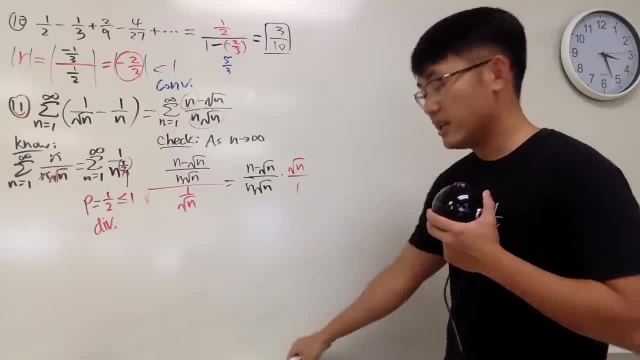 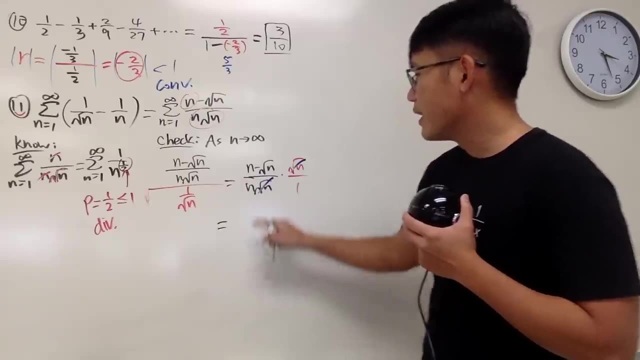 square root of n over 1 like this, And of course you can see that cancel, cancel. And now let's do some more algebra. So still equal signs. We have n over n, minus square root of n over n, And. 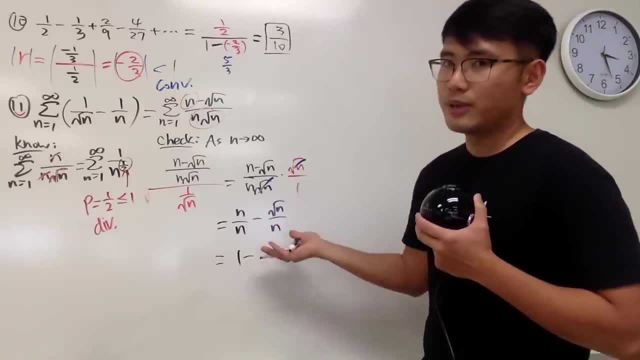 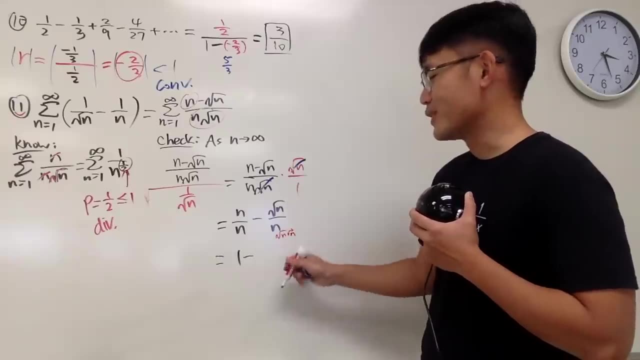 of course this is 1 minus and I'll show you guys how to cancel this the quick way. Look at n as square root of n, square root of n. So of course this is not cancel, So you have 1 over. 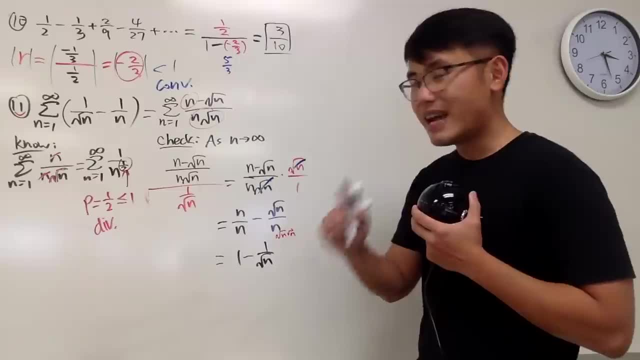 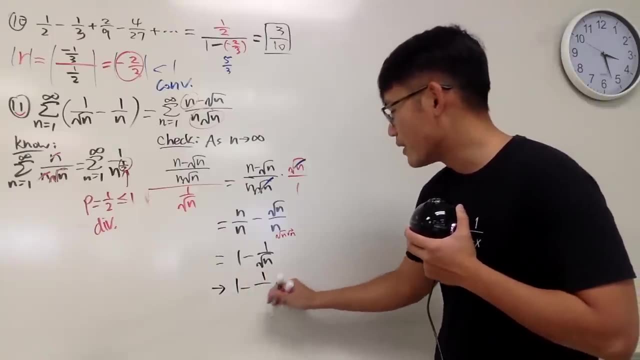 square root of n. Again, everything is just algebra now. Now we take the limit as n goes to infinity, So I'll just put down arrow for taking limit. This is 1 minus 1 over square root of infinity, which this part will. 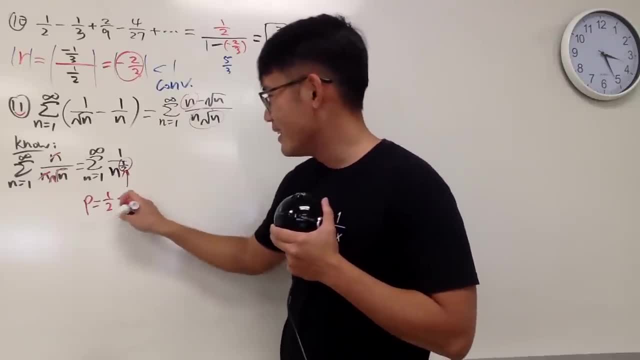 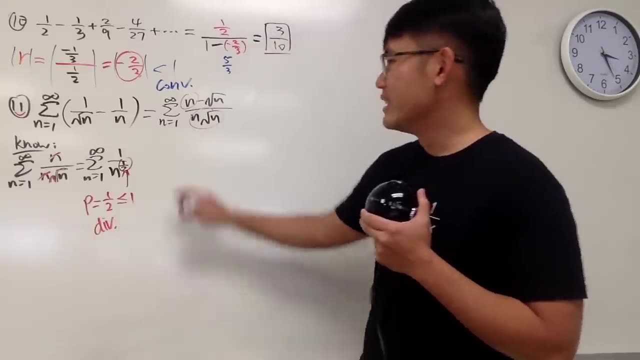 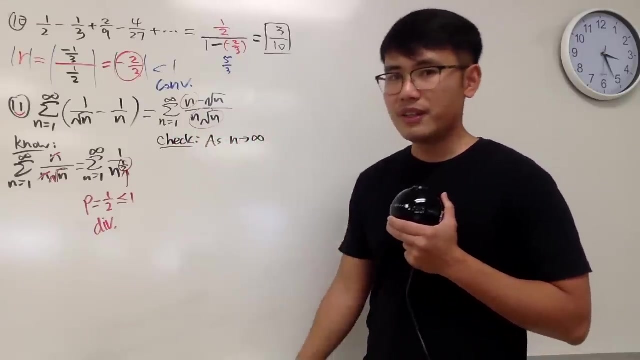 p is less than or equal to 1.. That's the p series test, And this, right here, diverges. Now we are going to do the check. Well, we take the limit as n goes to infinity. Put down the one that you want to work out. 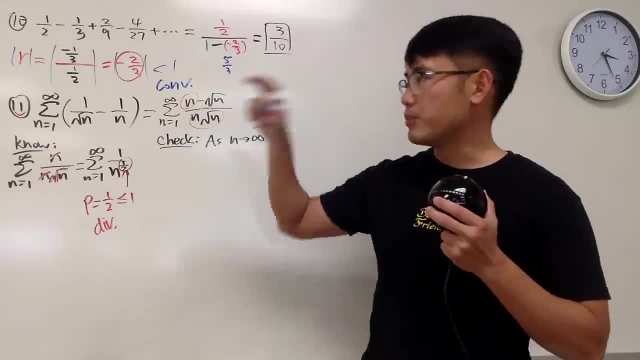 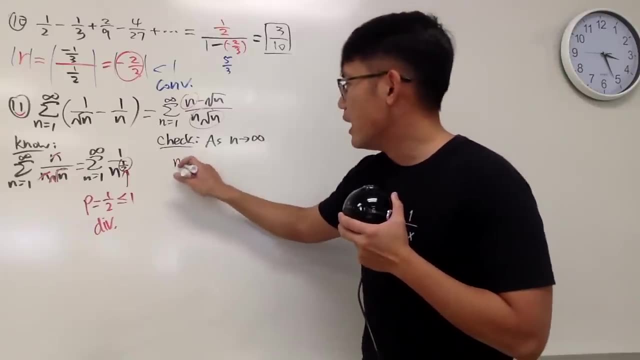 on the top right. And the truth is it doesn't really matter. You can put this on the bottom as well if you like, but to be consistent, let's put this one on the top. So here we have n minus square root of. 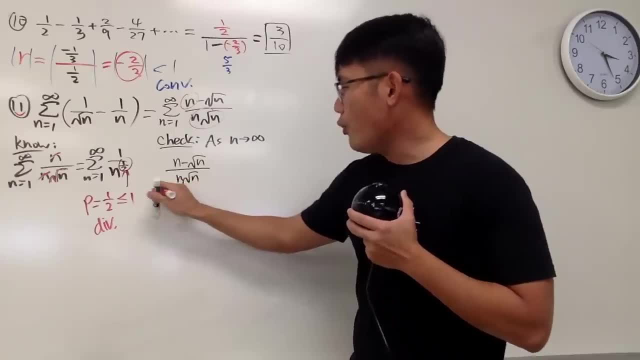 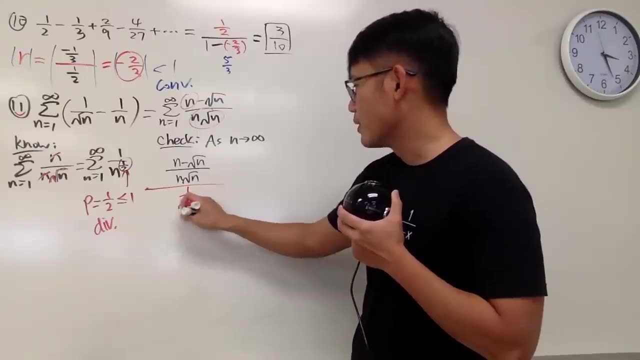 n over n, square root of n over. let me just put down over. let me put down 1 over square root of n, because everybody has a square root of n, so why not? So this is what we have Now do. algebra: Take this. 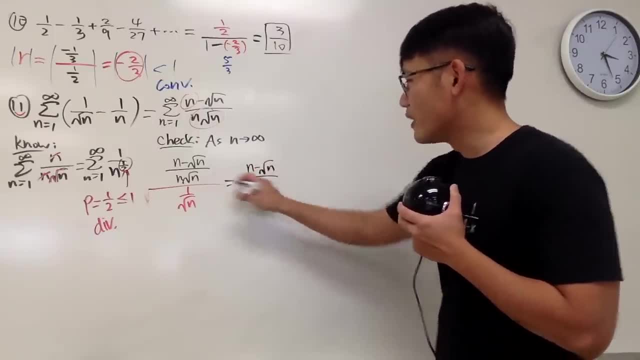 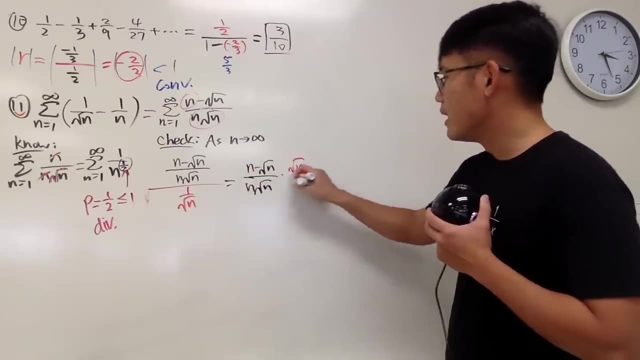 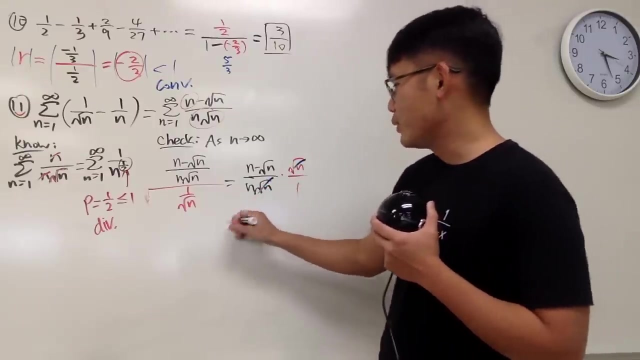 so we have n minus square root of n over n times square root of n, and we multiply by square root of n over 1, like this, And of course you can see that: cancel, cancel. And now let's do some more algebra. so still equal signs. 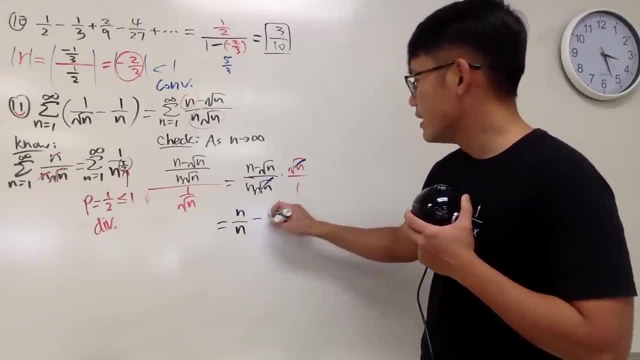 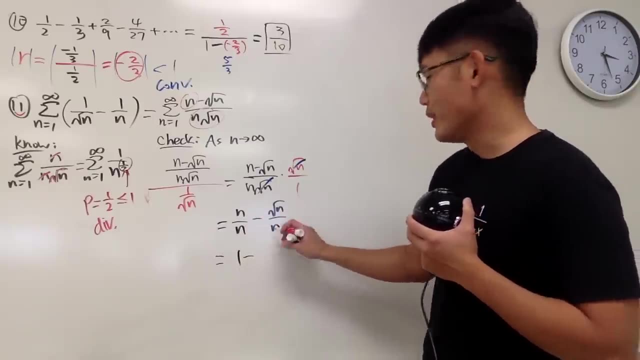 We have n over n, minus square root of n over n, And of course this is 1 minus, and I'll show you guys how to cancel this the quick way. Look at n as square root of n. square root of n. So of course this: 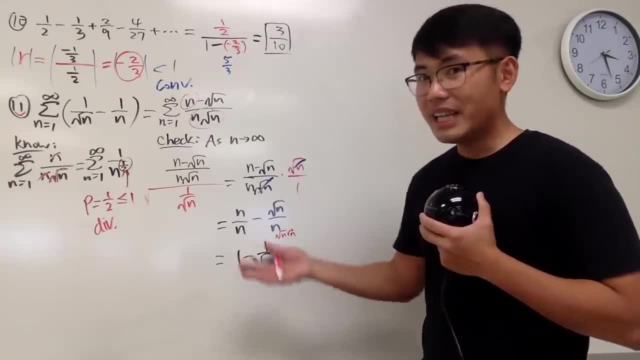 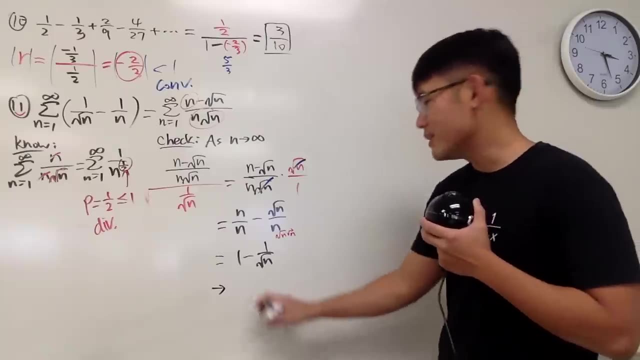 is not cancelled. so you have 1 over square root of n Again. everything is just algebra now. Now we take the limit as n goes to infinity. so I'll just put down arrow for taking limit. This is 1 minus. 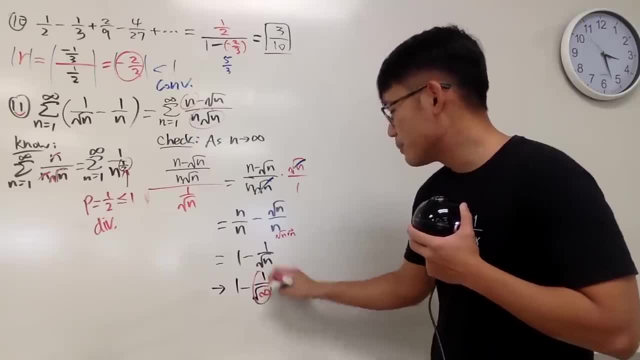 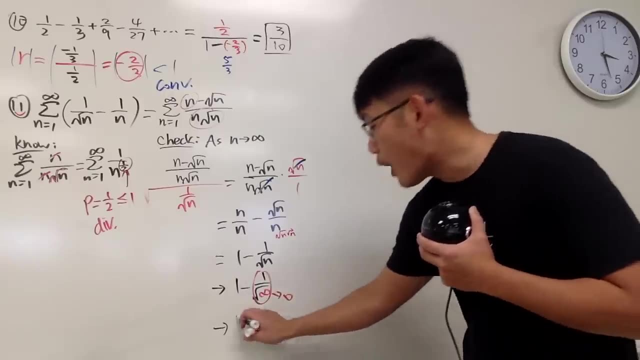 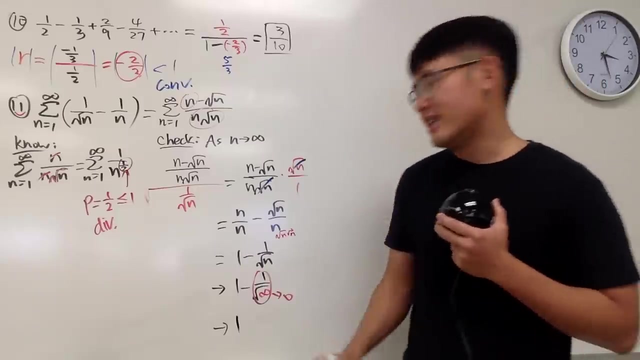 1 over square root of infinity, which this part will go to 0.. All in all this right here is just this: limit approaches 1.. Now for the limit completion test. can we use the 1?? Yes, we can, because 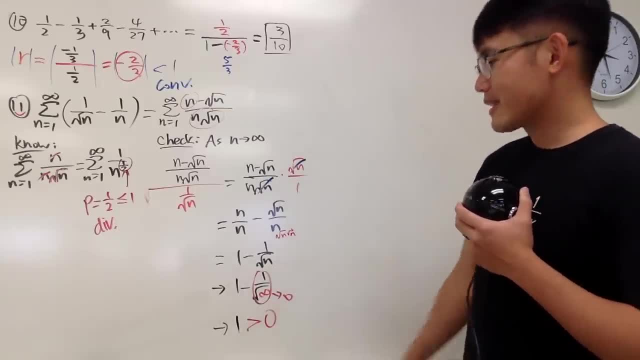 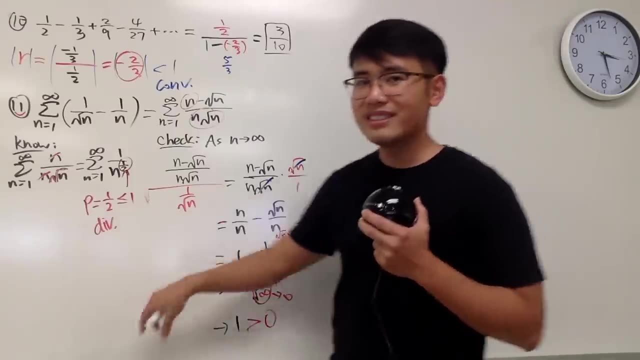 1 is greater than 0. Okay, Again, the idea is that this and that are pretty much of the same size. So if this right here diverges, this right here also diverges. So come back here. I will say: 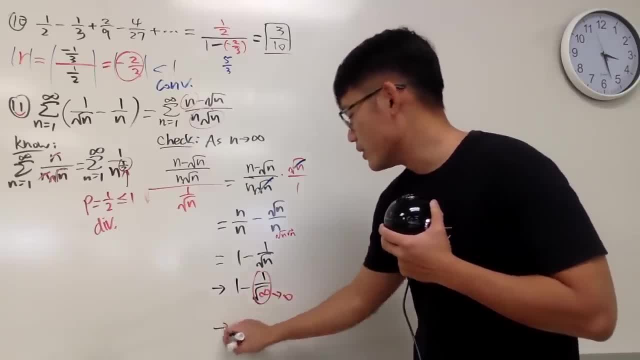 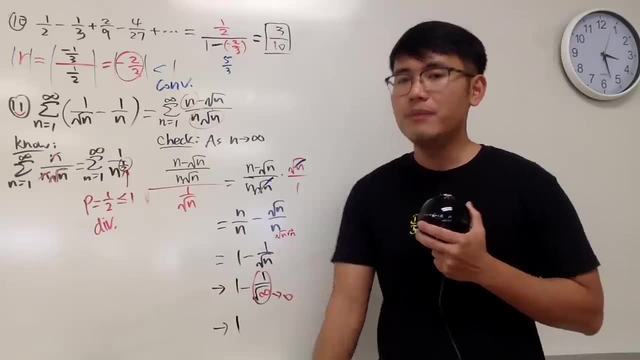 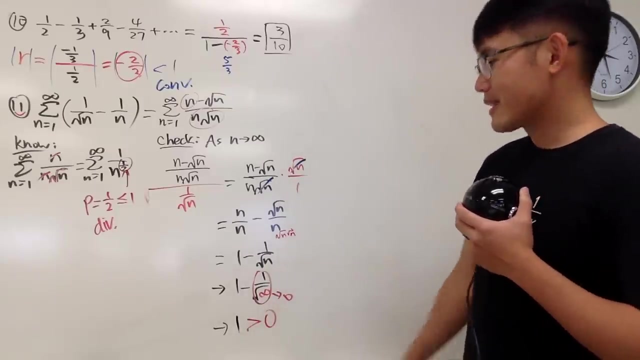 go to 0.. All in all, this right here is just this- limit approaches 1.. Now for the limit completion test. can we use the 1?? Yes, we can, because 1 is greater than 0. Okay. 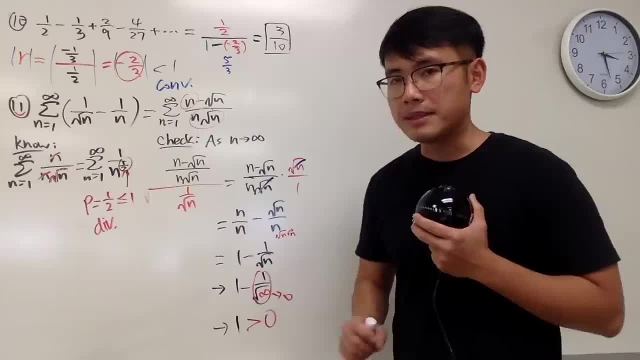 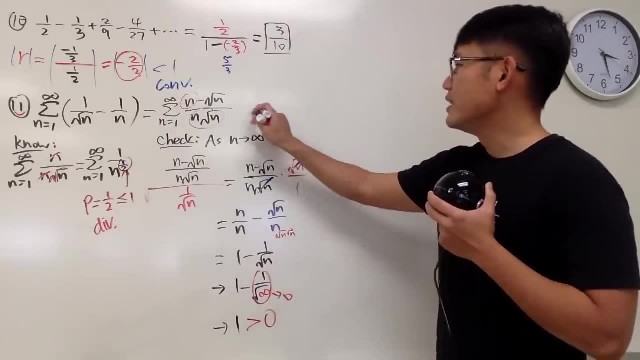 Again. the idea is that this and that are pretty much of the same size. So if this right here diverges, this right here also diverges. So come back here. I will say: this right here diverges as well. by we did the limit. 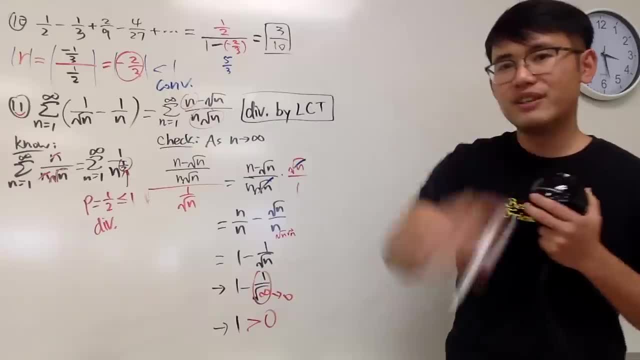 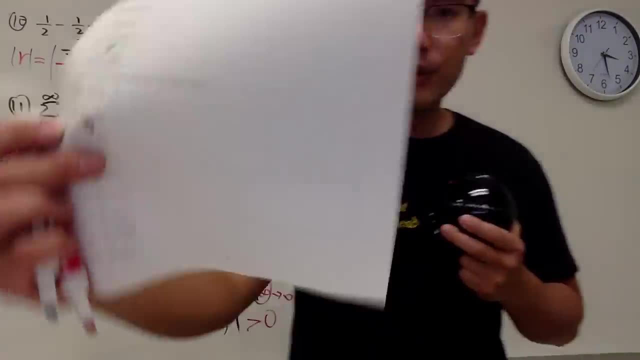 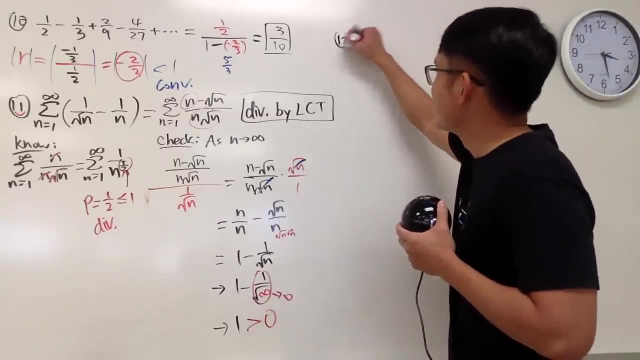 so this is the limit completion test. L C, T for that Done Cool. Now moving on to question number 12.. Right here the sum. oh my god. the natural log question again. Oh my god, who did that? 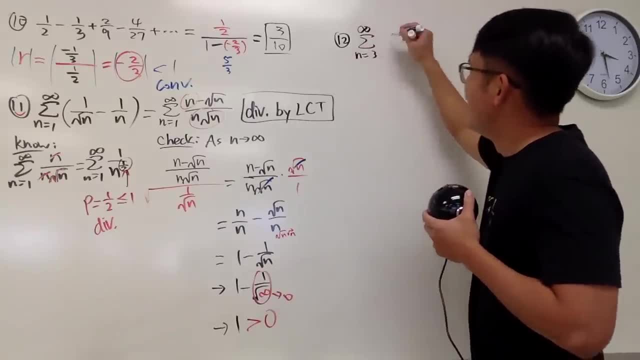 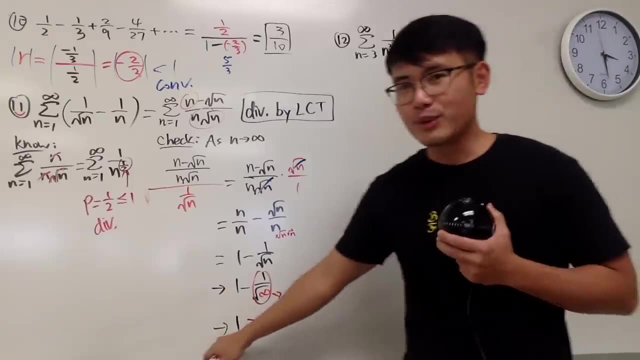 Yes, it's me Anyway. 1 over n square ln n. By the way, a lot of these questions are really popular test questions. okay, A lot of questions are the questions that you should know. I will have to admit some of the questions. 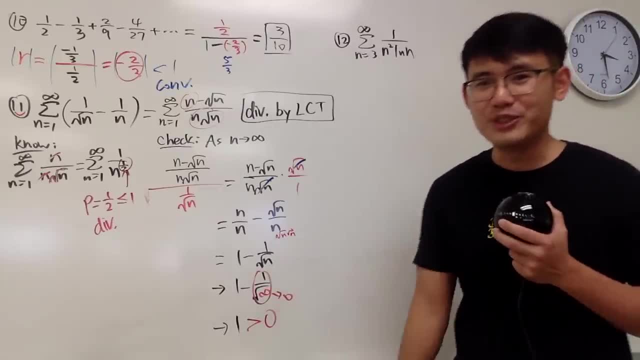 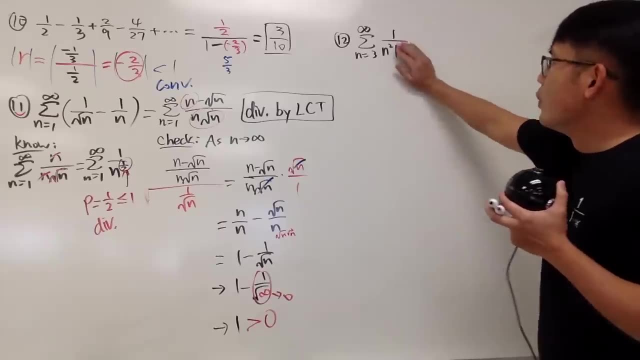 I created is for fun, so hopefully you guys will really enjoy it. this I don't know how many hours video. Anyway, here we go. Here's a small part: 1 over n square the series, for that it converges. 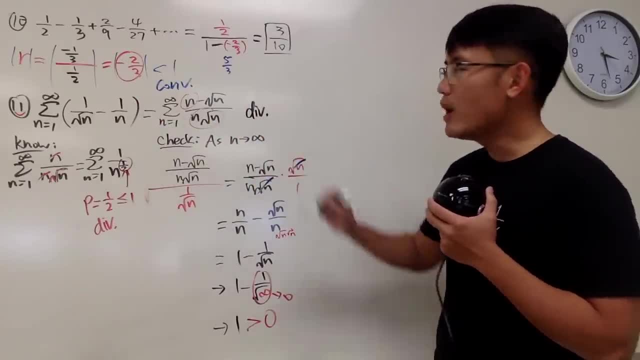 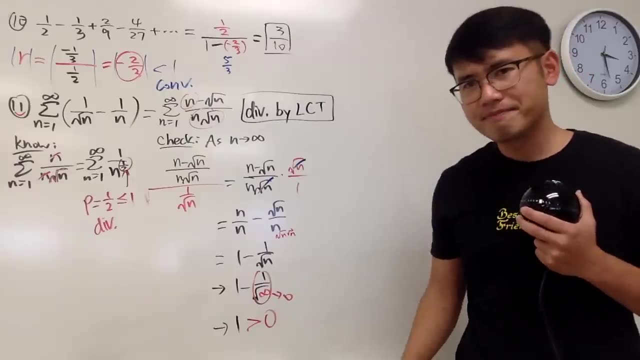 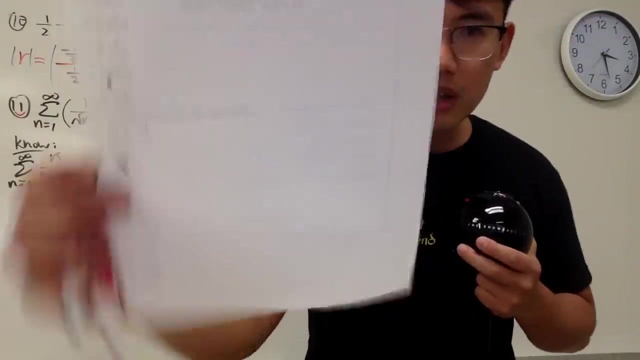 this right here diverges as well by: we did the limit, so this is the limit. completion test: L, C, T for that Done Cool. Now, moving on to question number 12, right here, the sum. oh my god. 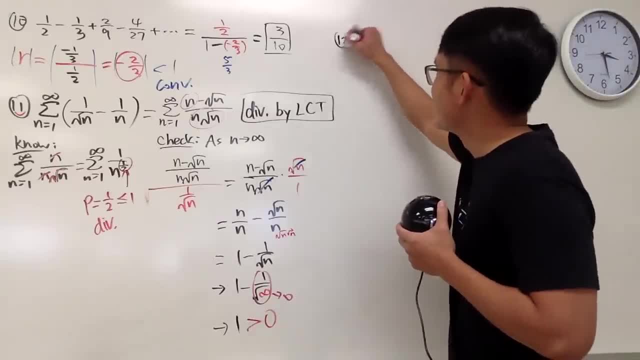 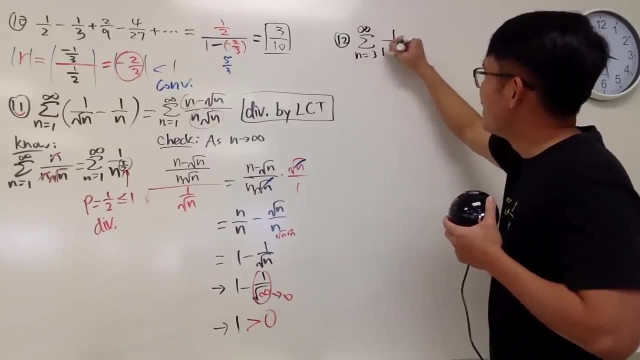 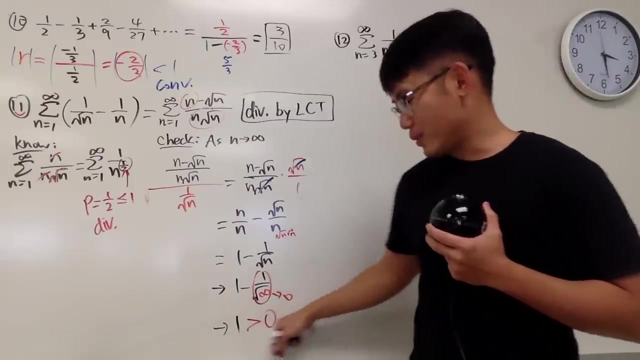 the natural log question again. Oh, my god, who did that? Yes, it's me Anyway. 1 over n squared ln n. By the way, a lot of these questions are really popular test questions. okay, A lot of questions are the questions. 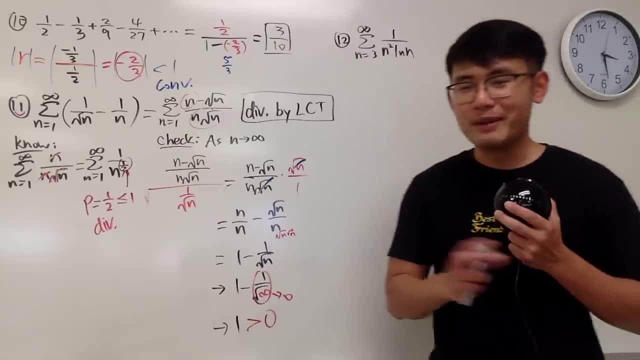 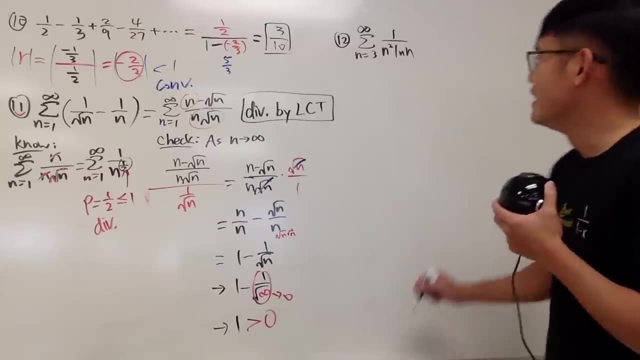 that you should know. I will have to admit some of the questions I'm I created so it's for fun, so hopefully you guys will really enjoy this. I don't know how many hours video. Anyway, here we go. 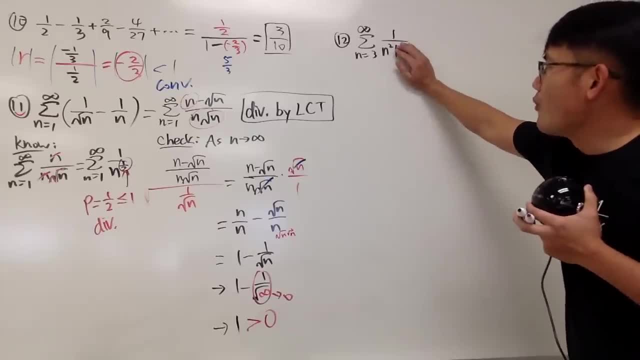 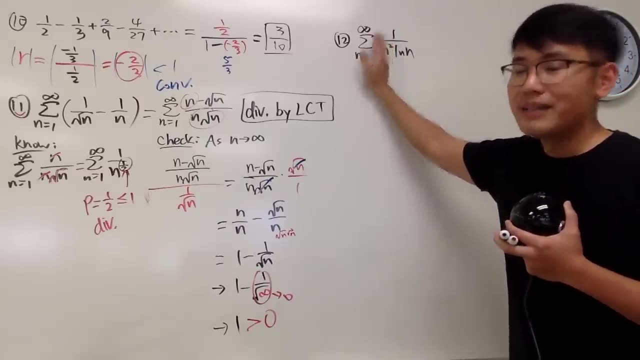 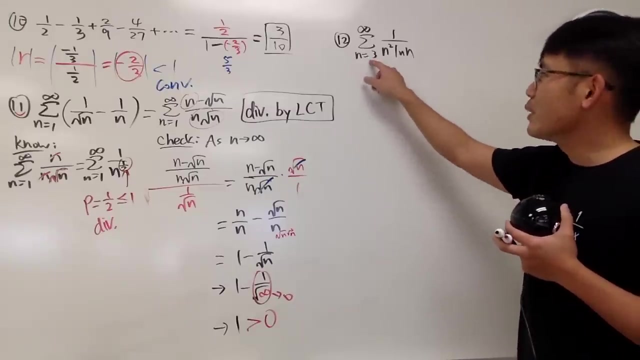 Here's a small part. 1 over n: squared the series for that it converges. 1 over ln n it diverges. Why? We did that already a few times all that time. Hmm, Check this out. n goes from 3. 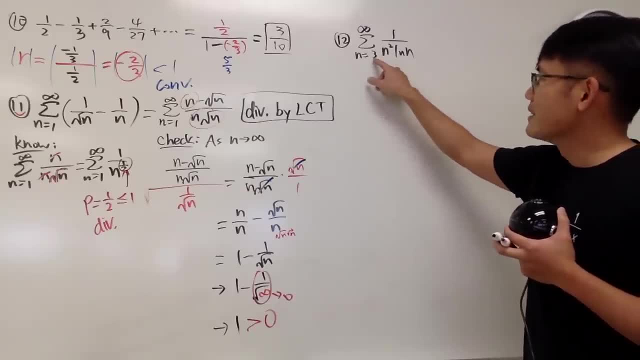 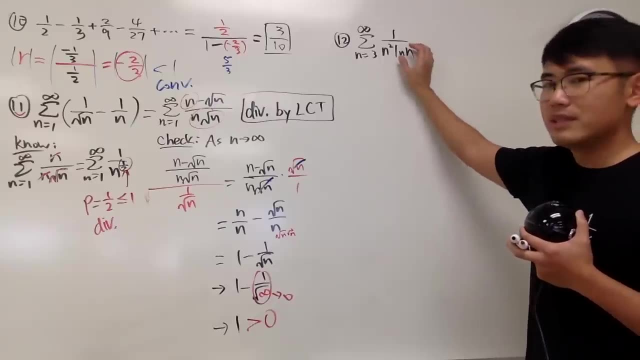 to infinity. okay, In fact, when n is 3, ln 3,, which is bigger than ln e, which is 1, so the bottom is going to be bigger than 1 for this part, If you put this away. 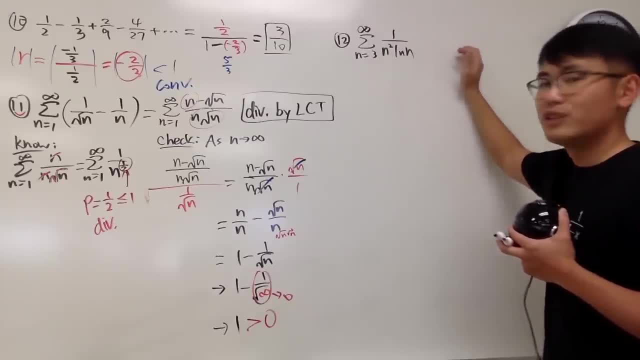 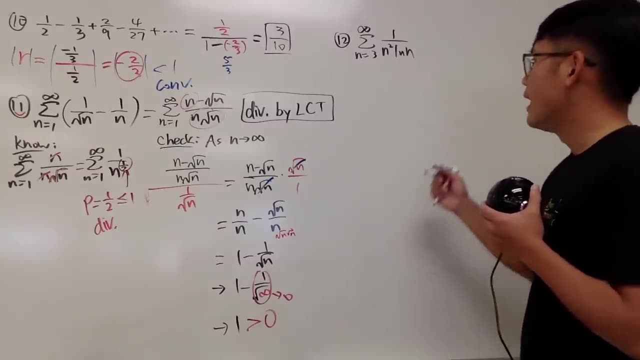 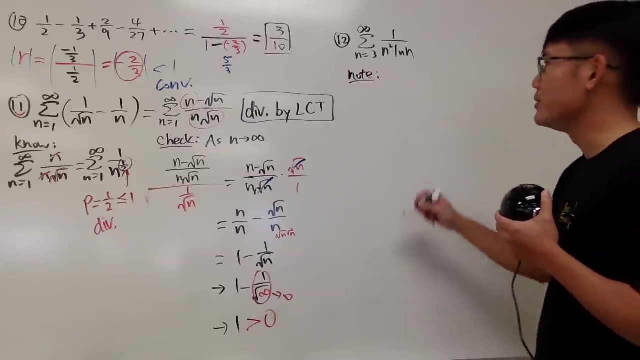 you can get this to be less than the sum as 1 over n squared Converges, nicely. So here is the deal. I will just put this down, just tell you guys, Note, we can put the answer up to you. 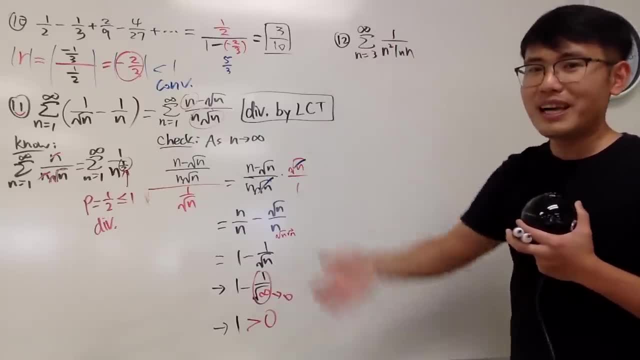 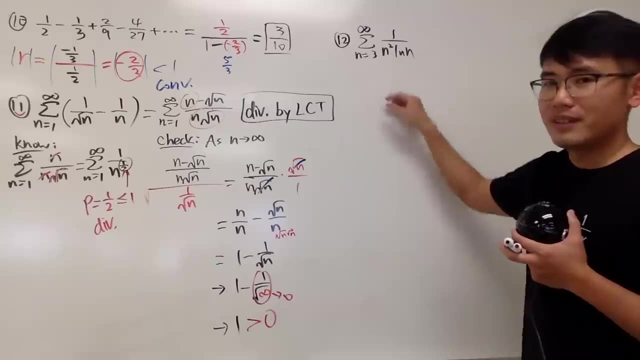 1 over ln n. it diverges Why We did that already a few times all that time. Huh, Check this out. n goes from 3 to infinity. okay, In fact, when n is 3, ln 3,. 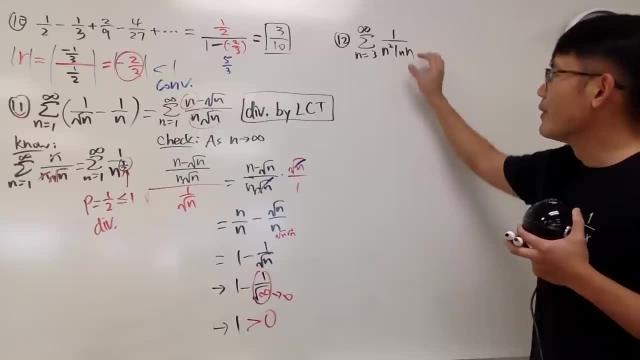 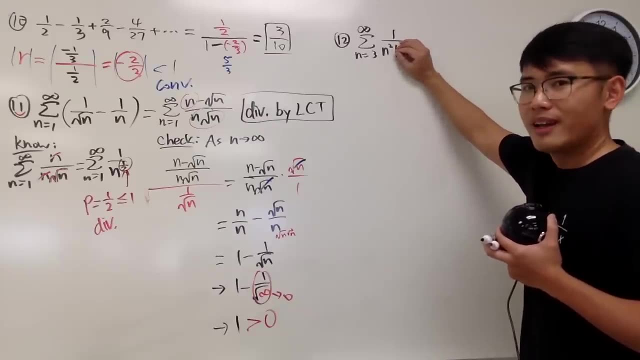 which is bigger than ln, e, which is 1.. So the bottom is going to be bigger than 1 for this part. If you put this away, you can get this to be less than the sum as 1 over n square converges. 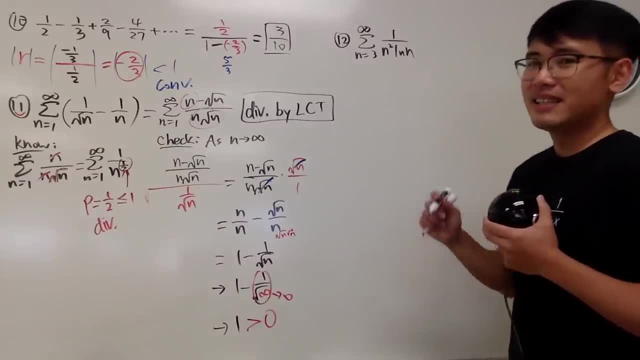 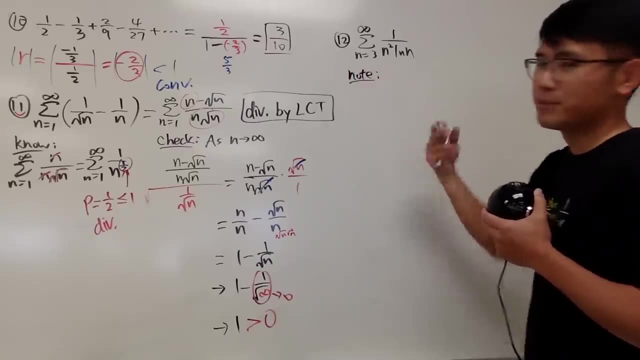 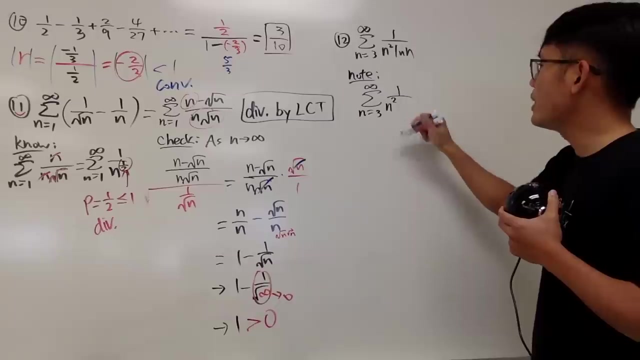 nicely. So here is the deal. I will just put this down. just tell you guys, Note, we can put the answer up to you. Note: the sum as n goes from 3 to infinity, 1 over n square. 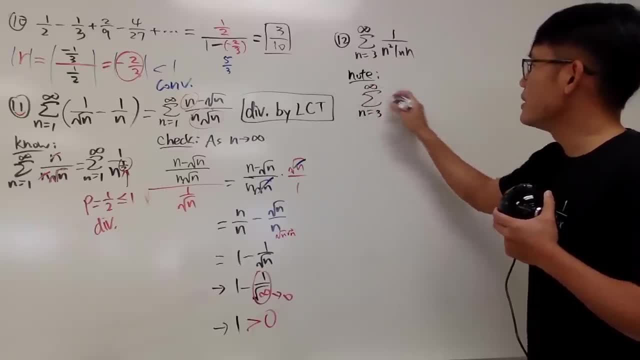 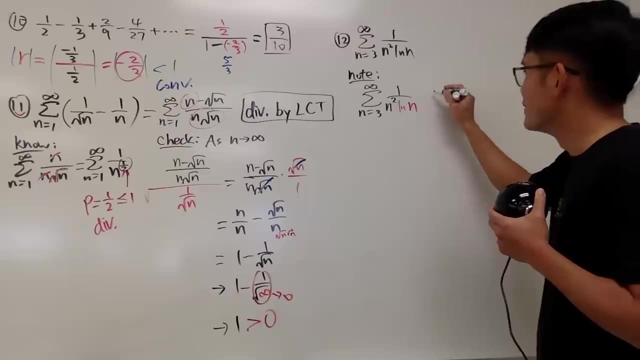 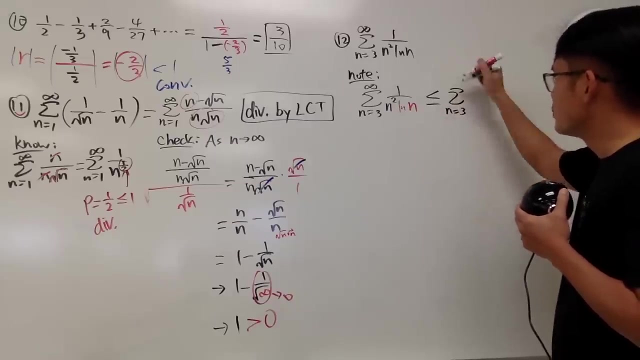 Note the sum as n goes from 3 to infinity. 1 over n squared ln n. right here I'm about to replace this, So I'm going to say this is actually less than or equal to the sum as n equals 1, I mean 3 to infinity. 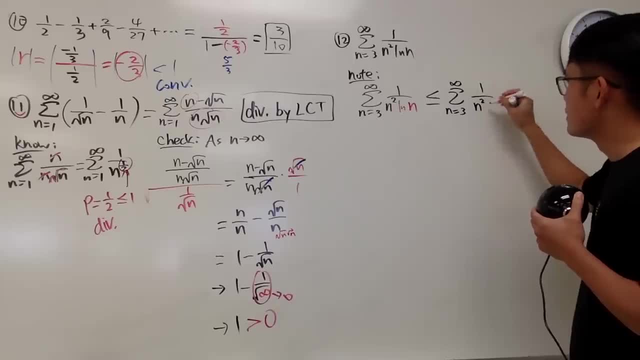 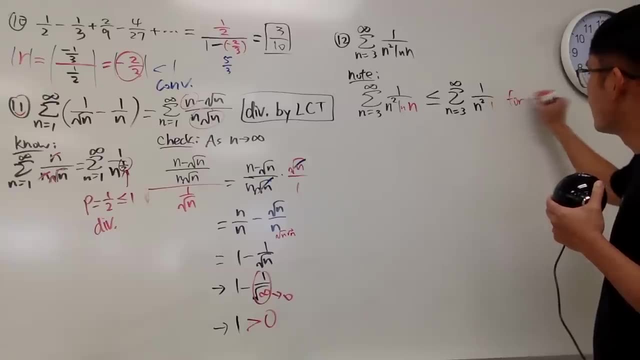 1 over n to the second power times: 1,. pretty much You don't have to mention the 1, it doesn't really matter. And the deal is that this is true for n is greater than or equal to 3.. Technically, 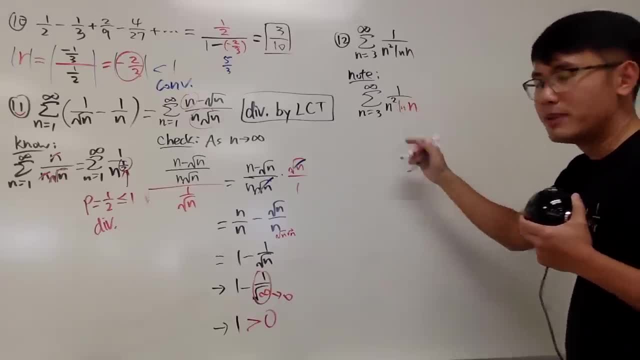 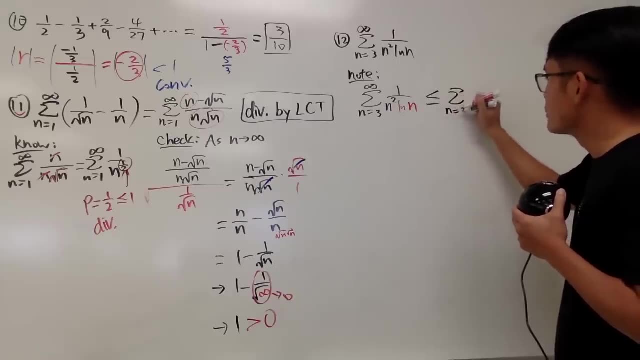 ln n. right here I'm about to replace this, So I'm going to say this is actually less than or equal to the sum, as n equals 1, I mean 3 to infinity, 1 over n to the second power. 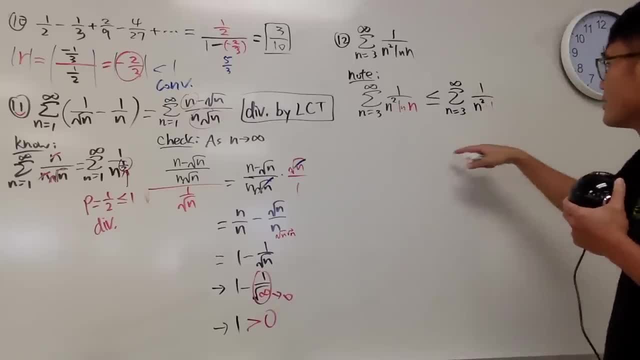 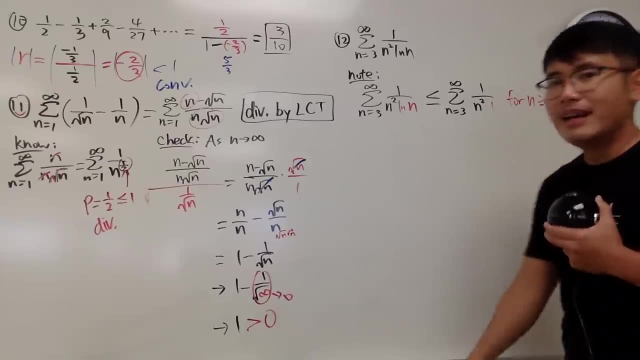 times 1,. pretty much You don't have to mention the 1,, it doesn't really matter. And the deal is that this is true for n is greater than or equal to 3.. Technically, when you have 2,. 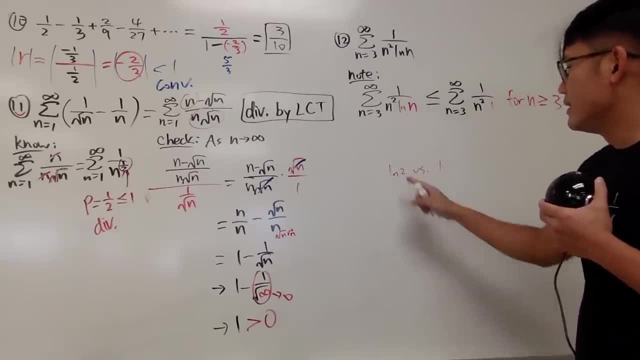 ln 2 versus 1, this is smaller than that. So if you do the reciprocal 1 over ln 2, it's actually bigger than 1, right, But again, that's why I start with 3, so that I can. 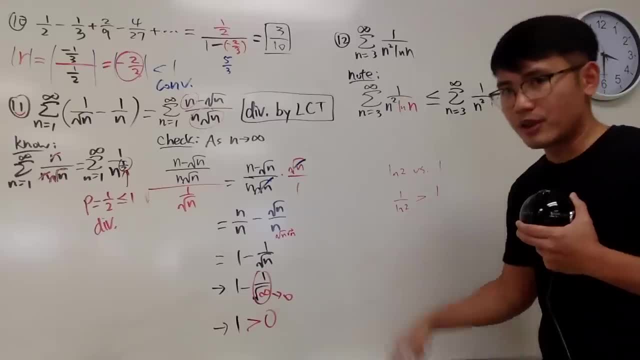 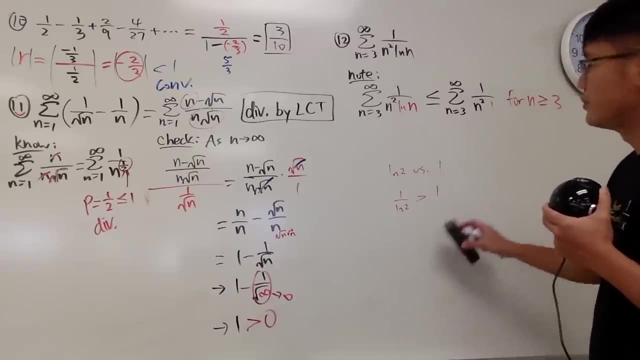 say this statement easily, okay, So I don't want to talk about the things that cause unnecessary confusion, especially if you're doing this for the first time, So I start with 3.. Okay, So, as you can see this right here now, 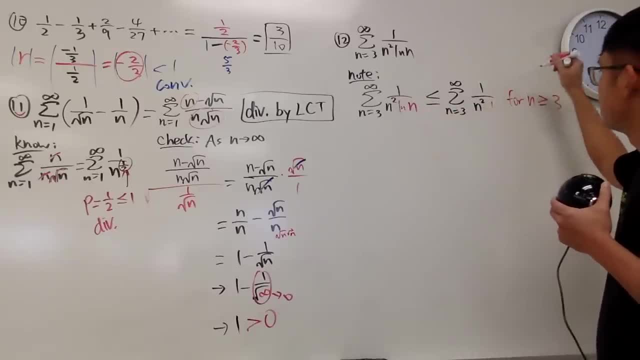 this is true because, again, we take this out. Yeah, I'll just say, since ln n is of course bigger than 1, right? Okay? so here again, let's put down: p is 2,, which is: 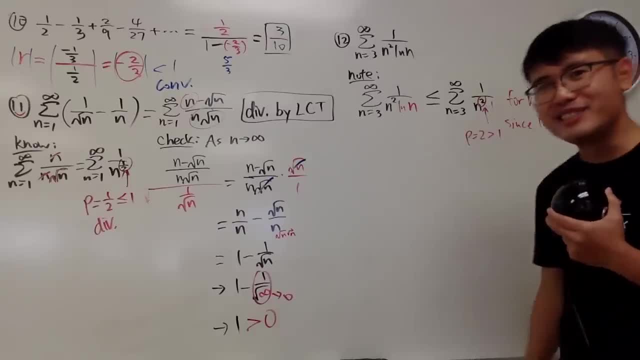 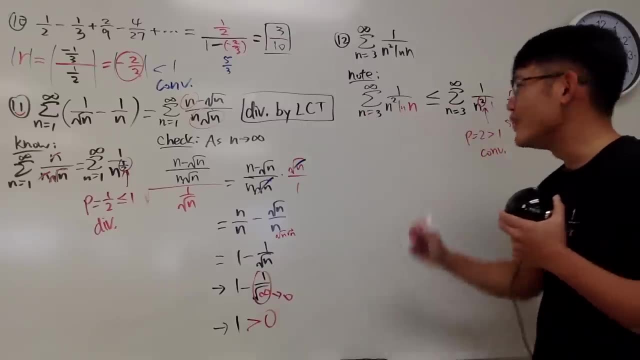 greater than 1, because we're using the p series, factor p series. maybe This right here converges. Well, this is less than a convergent, so we know this right here also converges. So now I'll just 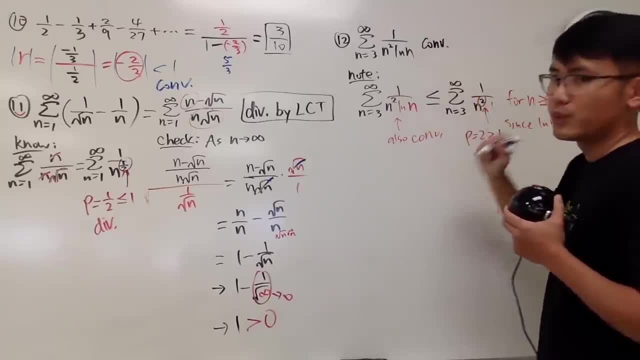 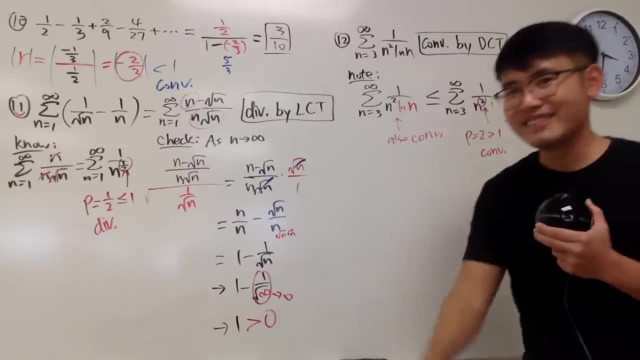 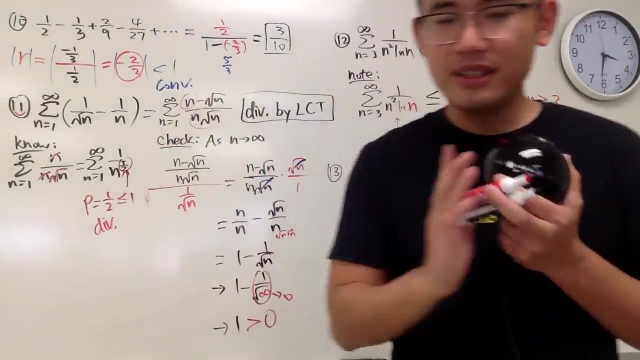 come back here and say this right here: Converges as well, Why? By the direct comparison test. And with that we are done. Right, Okay, number 13.. I feel like I like these markers more because my hands aren't dirty as the. 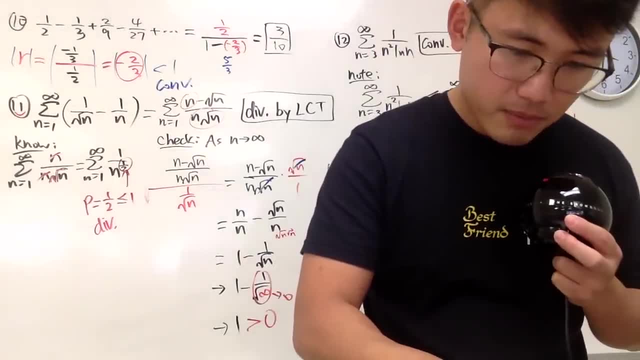 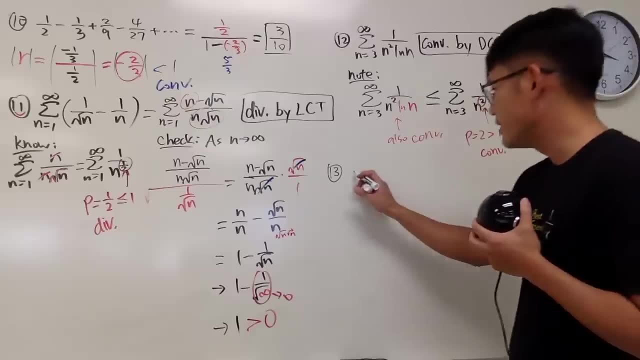 one that we had last time. Okay, okay, okay, Number 13 right here. I think I can be able to fit in that The sum as n goes from 1 to infinity, 1 over square root of n, e to the square root of n's. 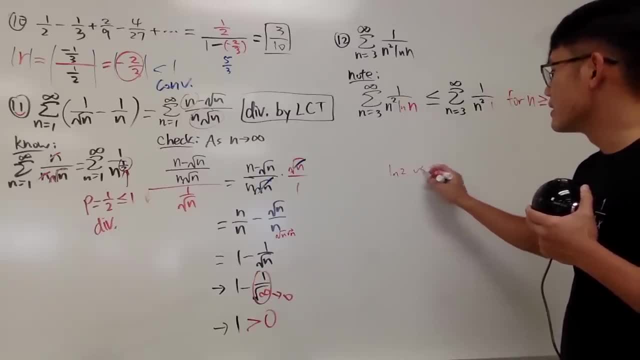 when you have 2, ln 2 versus 1, this is smaller than that. So if you do the reciprocal, 1 over ln 2 is actually bigger than 1, right, But again, that's why I start with 3, so that I can say: 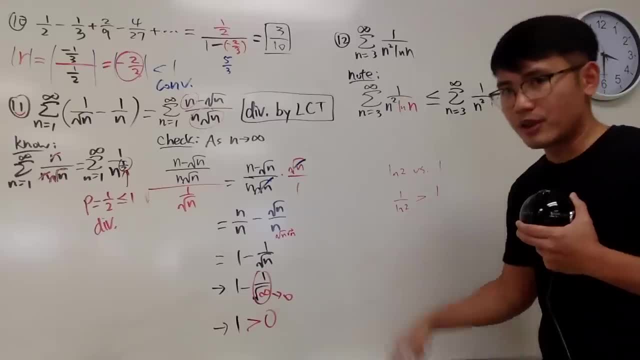 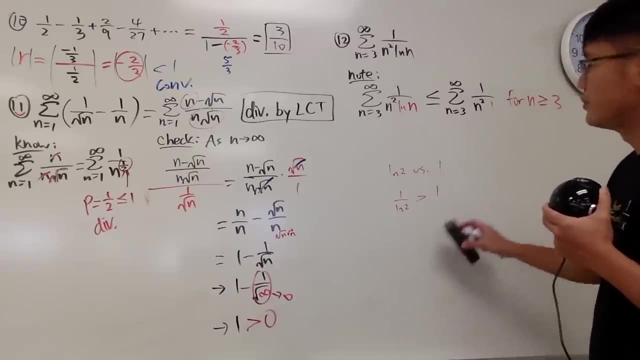 this statement easily, okay, So I don't want to talk about the things that cause unnecessary confusion, especially if you're doing this for the first time, So I'll start with 3. Okay, So, as you can see this right here now, 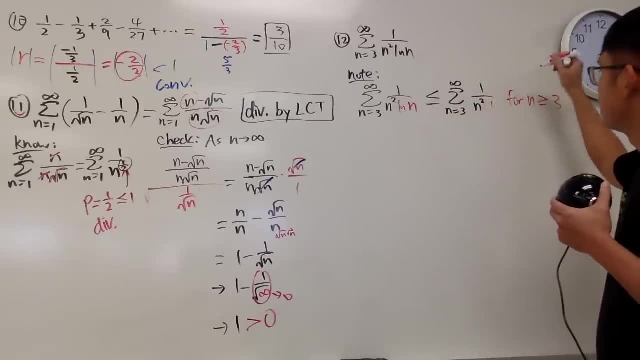 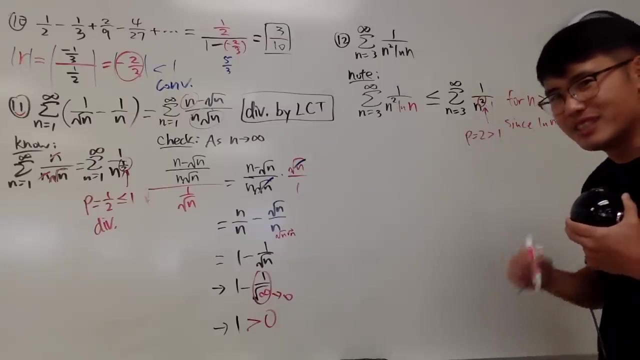 this is true because, again, we take this out. Yeah, I'll just say: since ln, n is of course bigger than 1, right, Okay? so here again, let's put down: p is 2, which is greater than 1, because we're using the. 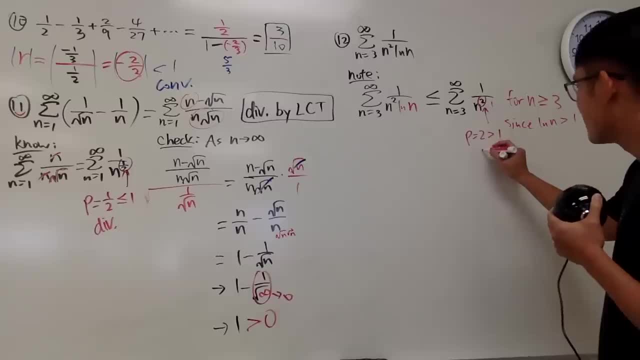 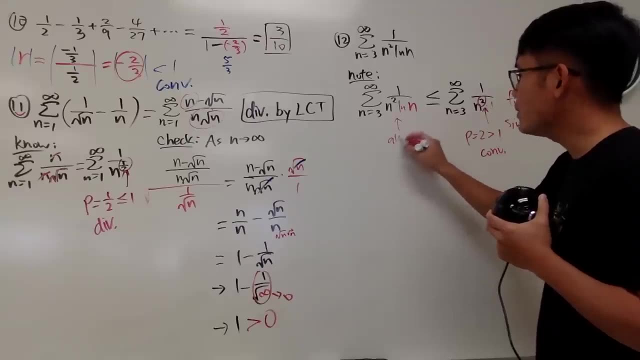 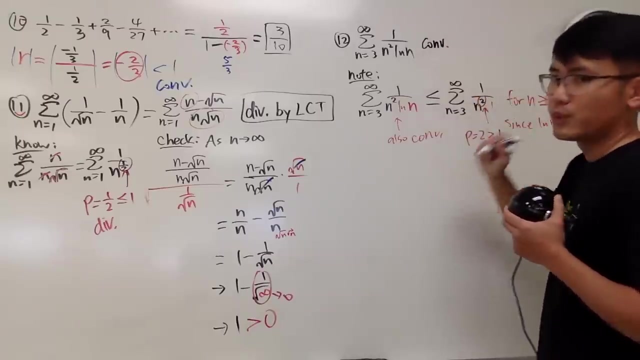 p-series, Dr P-series. maybe This right here converges. Well, this is less than a convergent. so we know, this right here also converges. So now I'll just come back here and say this right here converges as well. 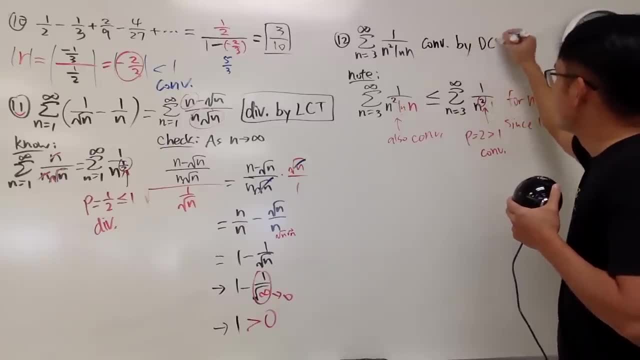 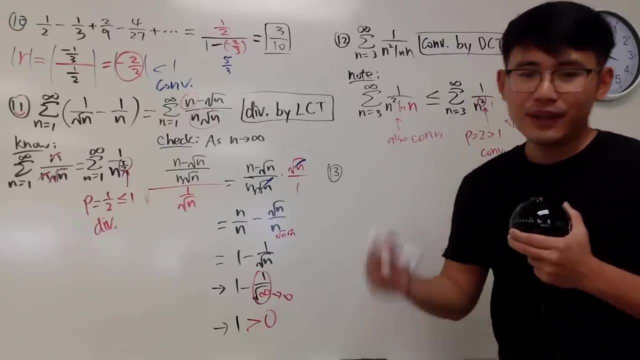 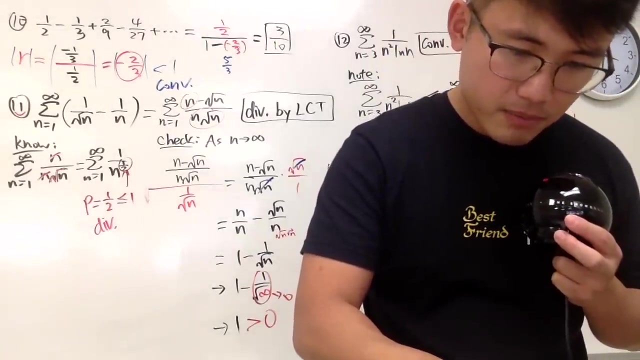 Why? By the direct comparison test. And with that we are done Right. Okay, number 13.. I feel like I like these markers more because my hands aren't dirty as the one that we had last time. Okay, okay, okay. 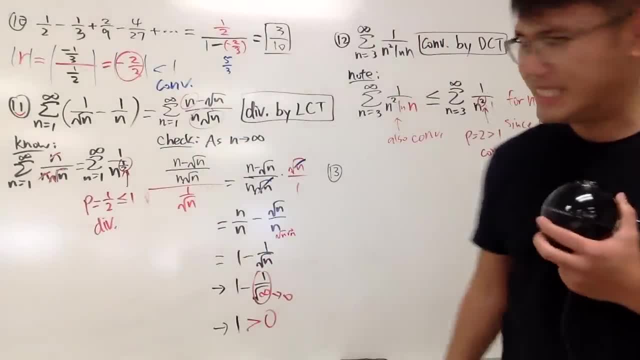 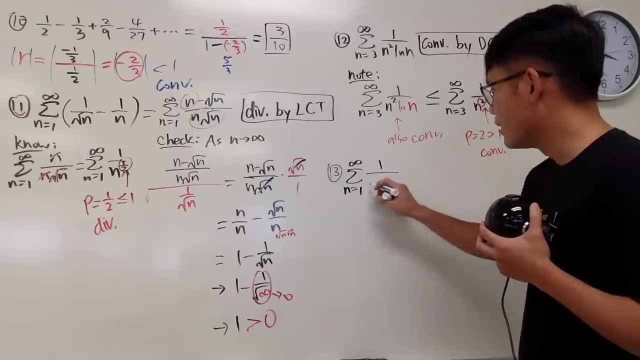 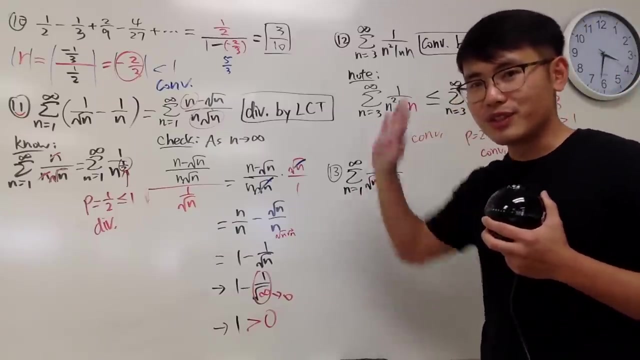 Number 13 right here I think I can be able to fit in that The sum as n goes from 1 to infinity, 1 over square root of n, e to the square root of n's power. like that. How many guests want to do integrals for this one? 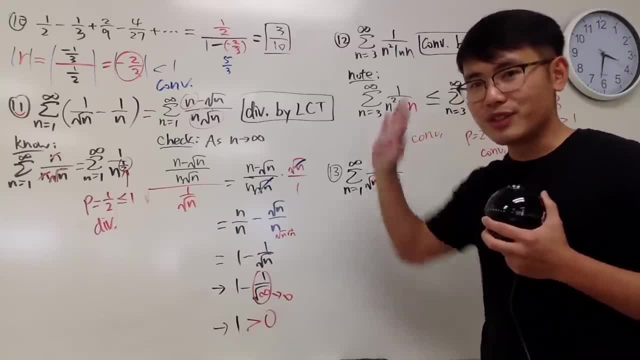 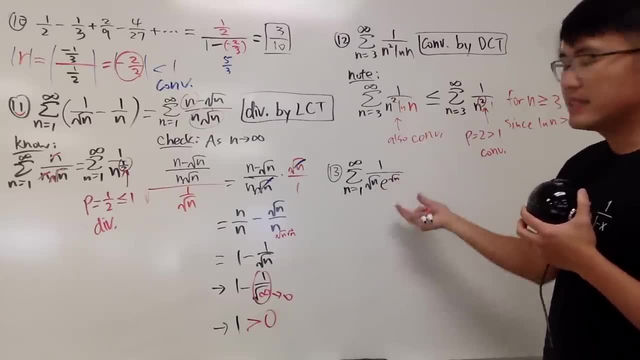 power like that. How many of you guys want to do integrals for this one? Technically you can. You had to mention 1 over square root of x. e to the square root of x. that's a positive decreasing function as x. 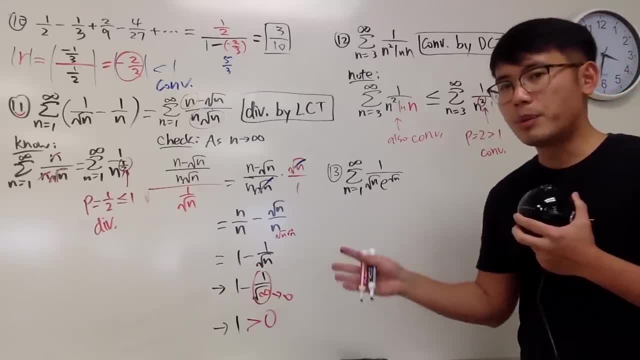 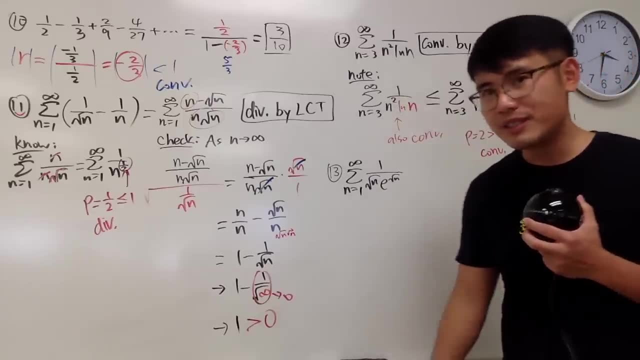 goes from 1 to infinity. You can just do the improper integral for that. but the deal is that you don't have to. let me show you how we can do it. Here is the deal. Here is the deal. Yes, if you just. 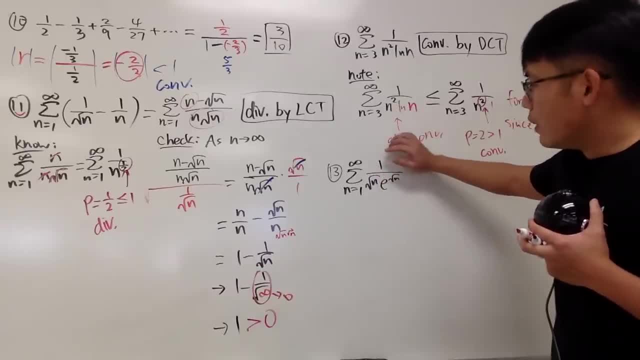 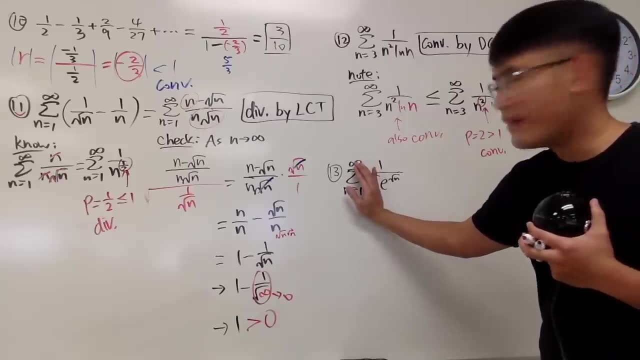 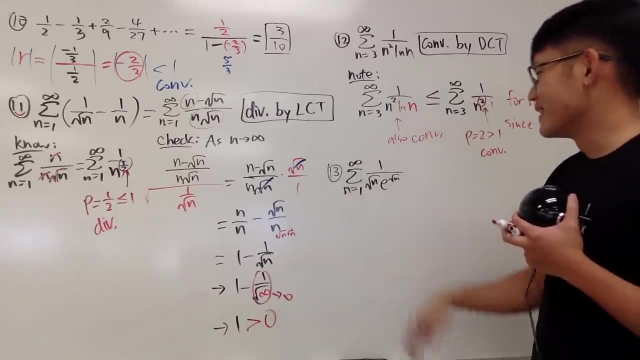 ignore this part. if you ignore this part, the sum of 1 over square root of n- it diverges. But if you look at this part- 1 over e to the square root of n- that actually converges, Because you. 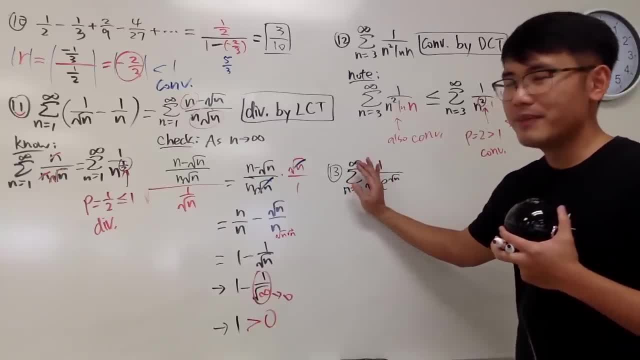 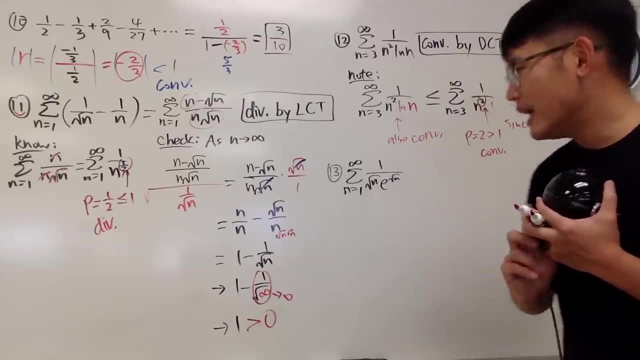 are about to see, of course, But the truth is this right here is actually a pretty big infinity right here, right, Even though you have the square root. that's bothering you, but it's actually doable. And again, for this kind of question. 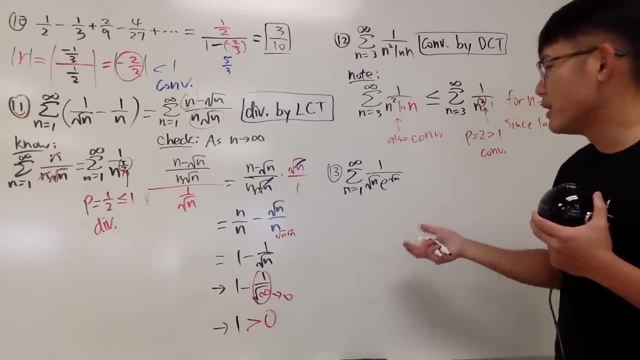 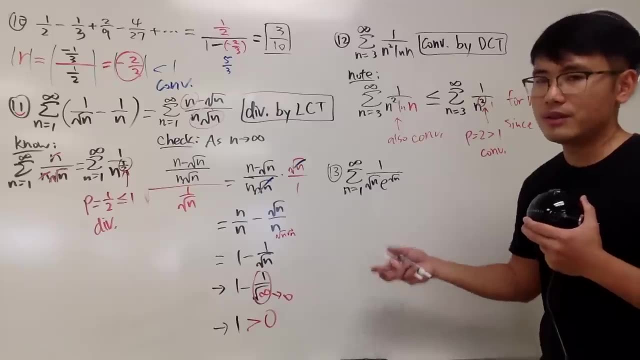 if I want to make it slightly more fair for my students, I will tell them hint. compare this with either the sum of 1 over n? square, or the sum of 1 over n, or 1 over square root of n. 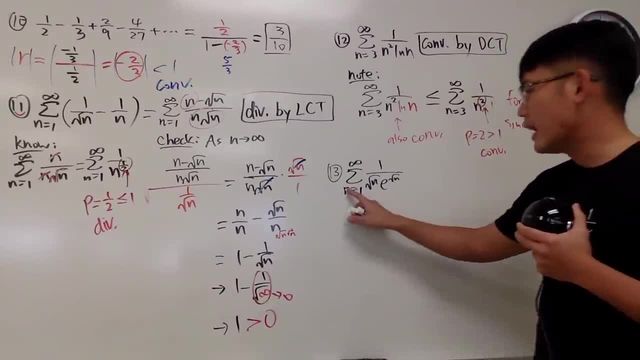 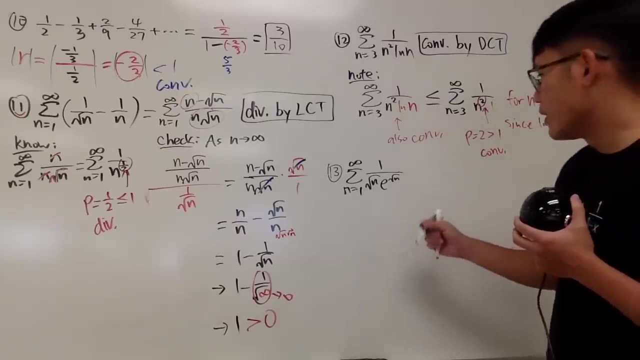 to see which one works, and all that. But I might provide a hint. So, my students, you have to watch my video, otherwise I will not do that for you guys, Alright, anyway. so let's see. how am I? 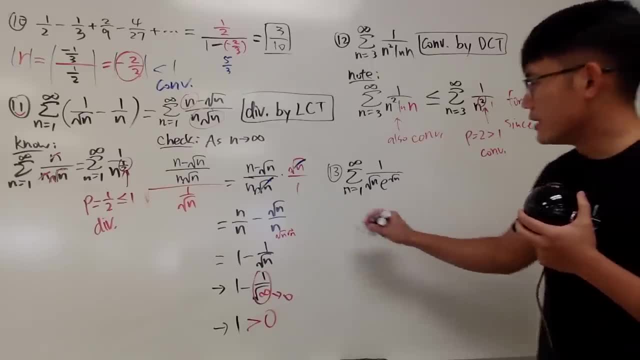 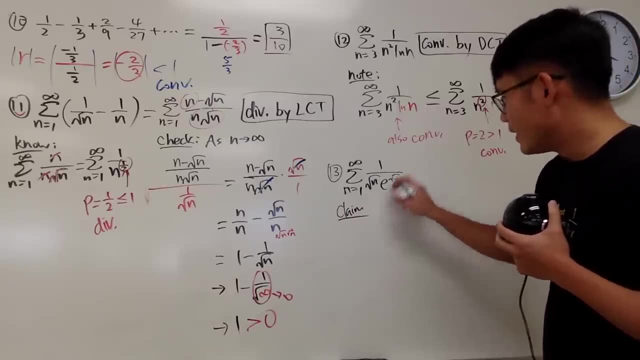 going to show you. Alright. so here is my claim. right, I'm going to claim that, Claim, Claim. I'm just going to look at this, part 1: over square root of n: e to the square root of n. I claim that: 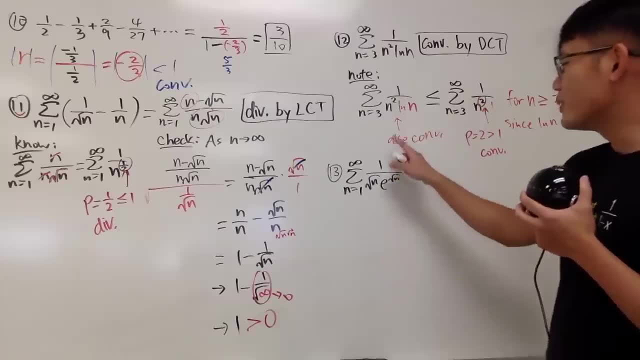 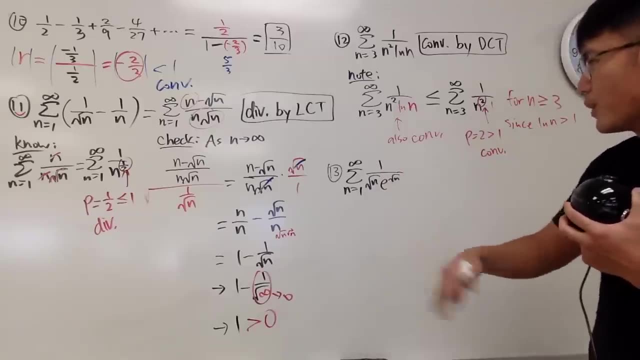 Technically you can. You have to mention 1 over square root of x, e to the square root of x. that's a positive decreasing function. as n. well, x, x goes from 1 to infinity. You can just do the improper integral. 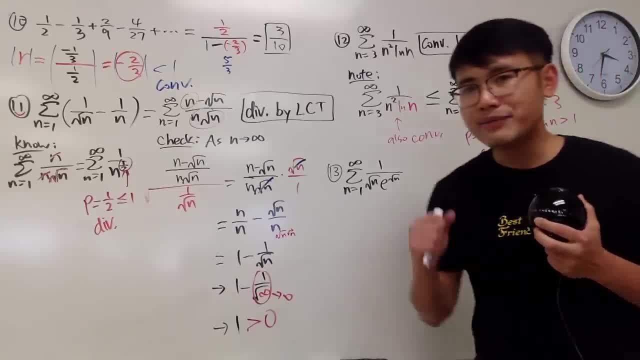 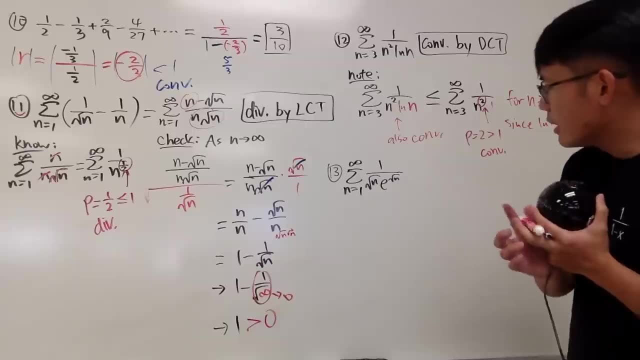 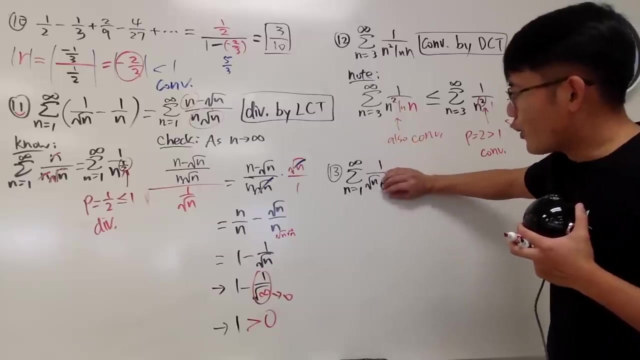 for that. but the deal is that you don't have to let me show you how we can do it. Here is the deal. Here is the deal. Yes, if you just ignore this part, if you ignore this part, the sum of 1 over 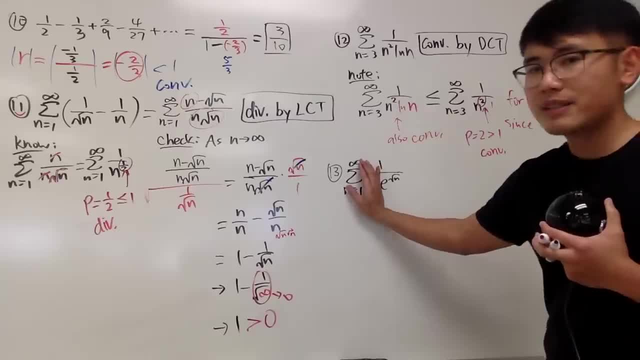 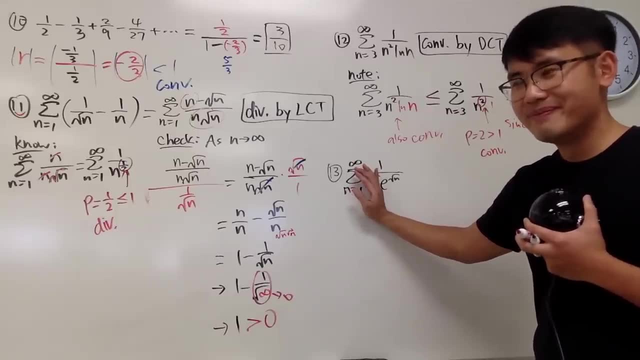 square root of n, it diverges. But if you look at this part, 1 over 1 over e to the square root of n, that actually converges, Because you are about to see, of course, But the truth is. 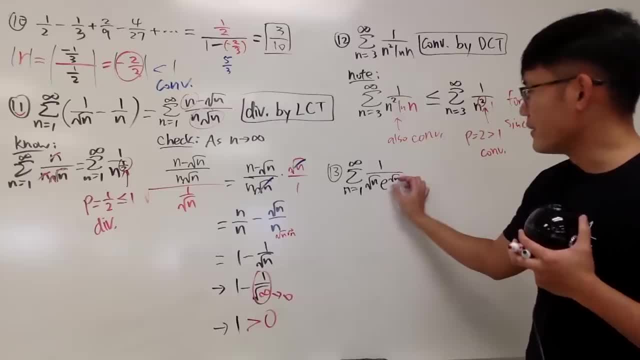 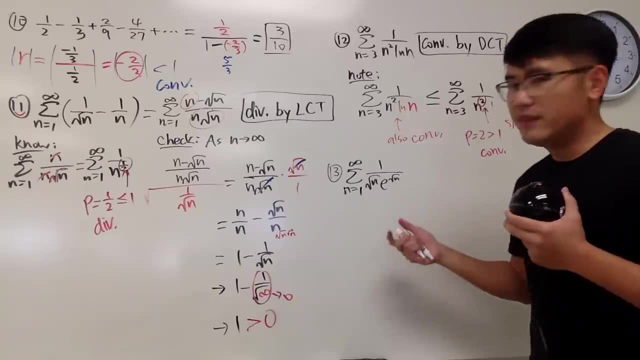 this right here is actually a pretty big infinity right here, right, Even though you have the square root. that's bothering you, but it's actually doable. And again for this kind of question, if I want to make it slightly more fair for my 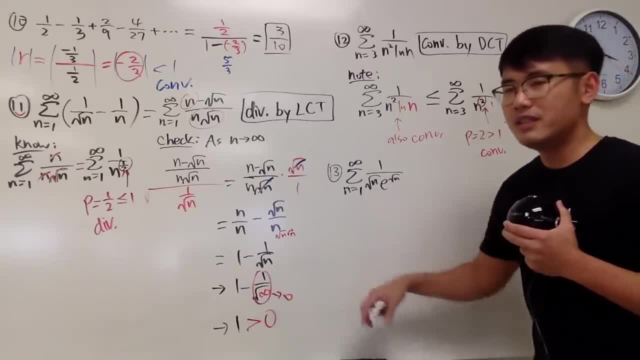 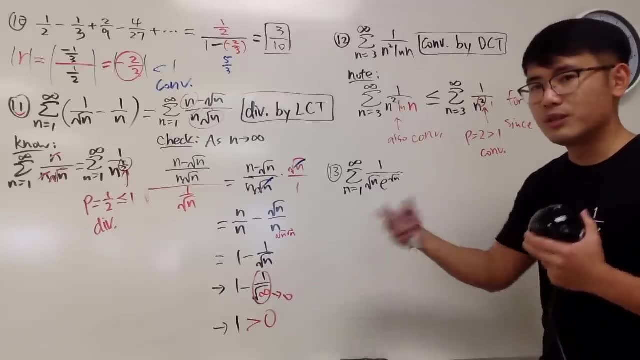 students. I will tell them hint: compare this with either the sum of 1 over n square, or the sum of 1 over n, or 1 over square root of n, to see which one works, and all that. But I have my profile. 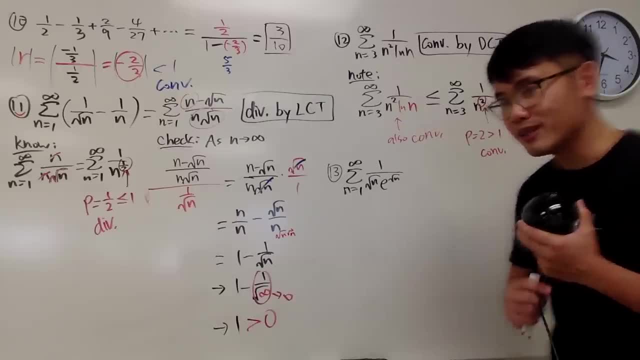 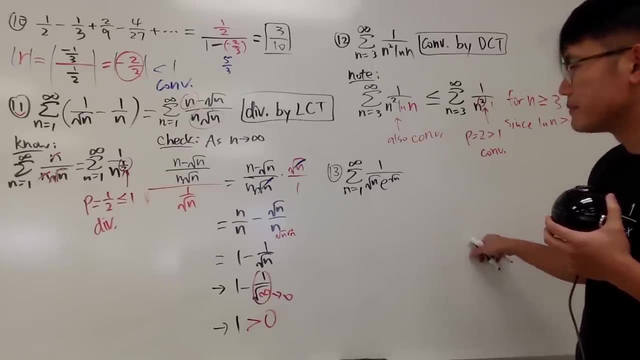 here, so my students have to watch my video, otherwise I will not do that for you guys, Alright, anyway. so let's see how am I going to show you? Alright, so here is my claim. right, I'm going to claim that. 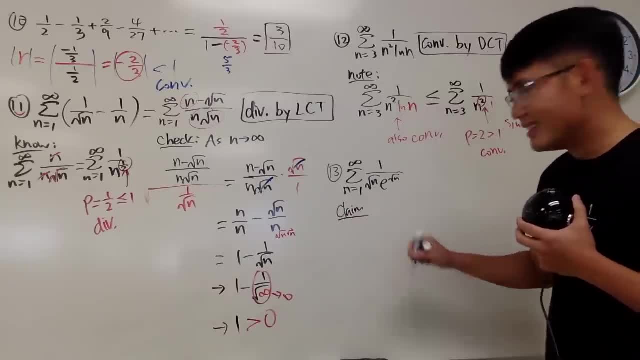 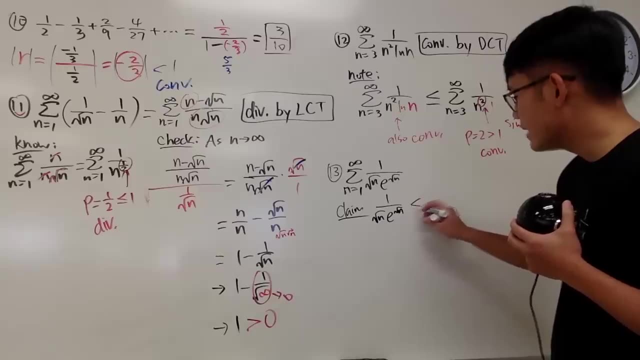 Claim, Claim. I'm just going to look at this part: 1 over square root of n. e to the square root of n. I claim that this, right here, is less than or equal to 1 over n squared, Because, again, 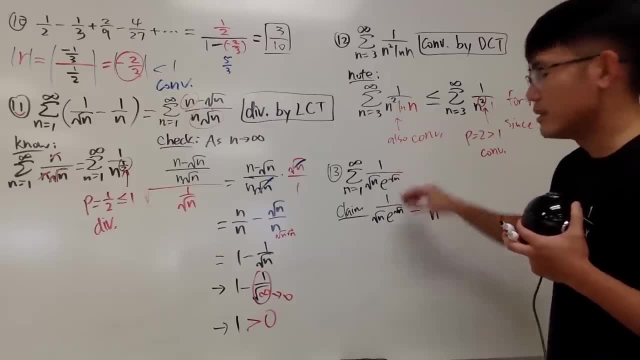 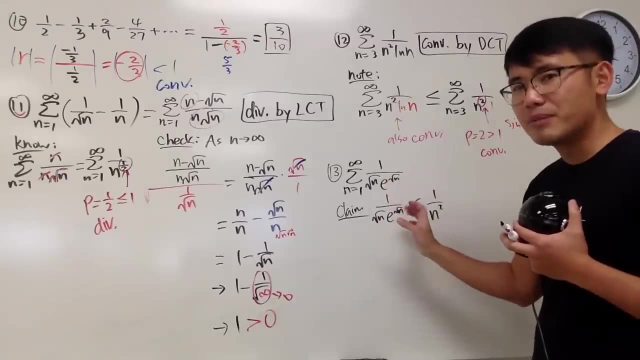 when we have e to something, this is not ln n, because e to the ln n is just n, so that would be bad. But e to the square root is pretty big infinity in the denominator, so I suspect that this right here converges. 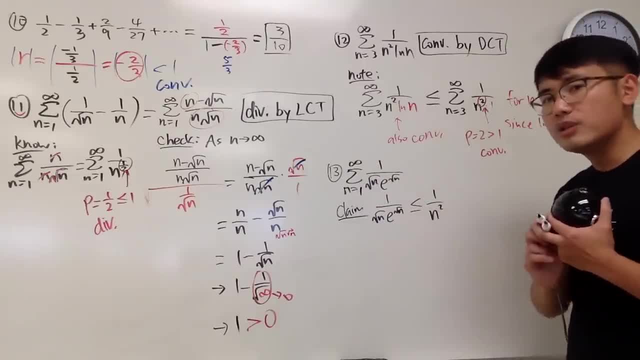 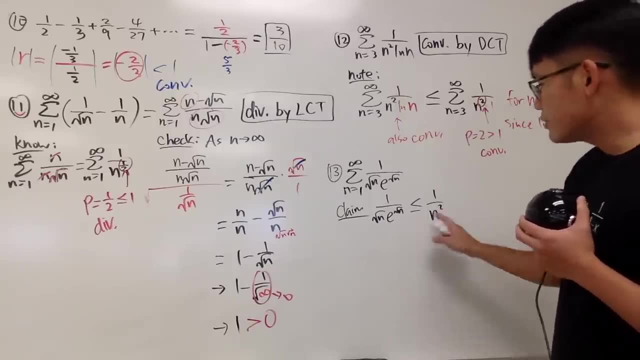 So I'm trying to compare this with a convergent and notice that I didn't put down the sum because I don't need to. I'm just trying to play around with this expression first. alright, So I claim this right here is true. 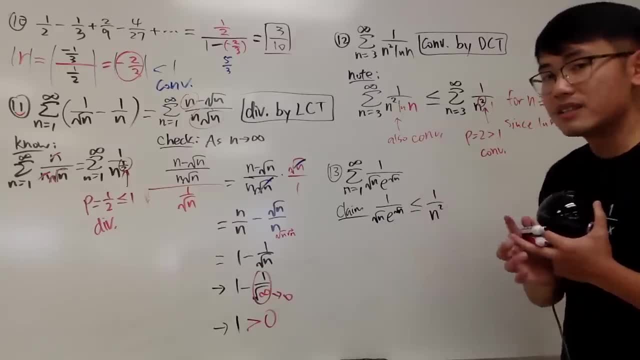 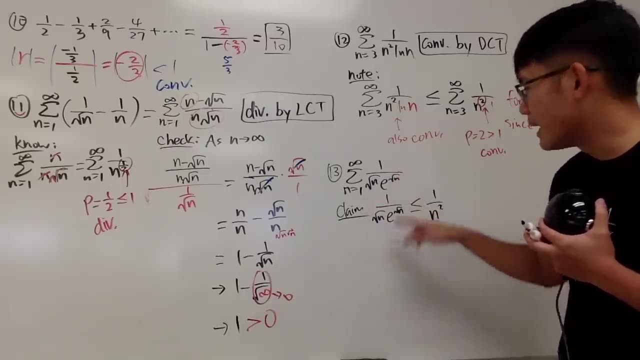 this right here is less than or equal to 1 over n squared, Because, again, when we have e to something, this is not ln and because e to the ln is just n. so that would be bad. But e to the square root. 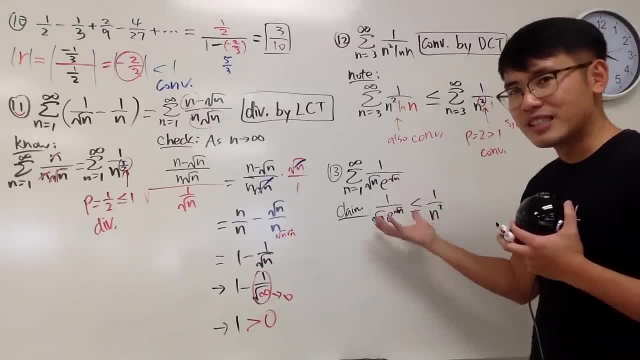 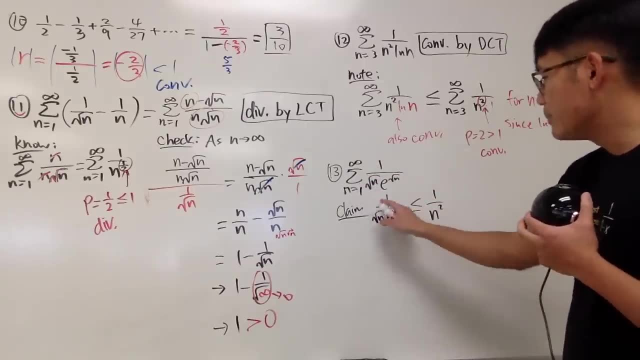 is pretty big infinity in the denominator, so I suspect that this right here converges. So I'm trying to compare this with a convergent and notice that I didn't put down the sum because I don't need to. I'm just trying to play around with this expression. 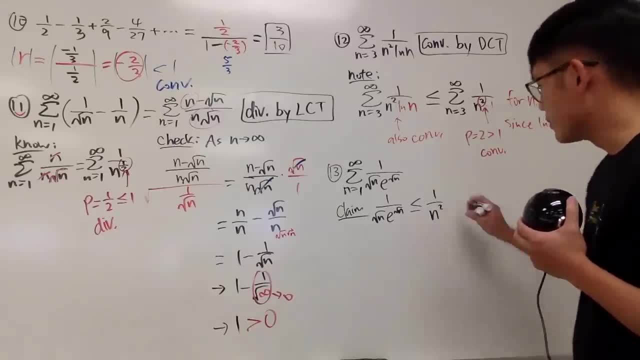 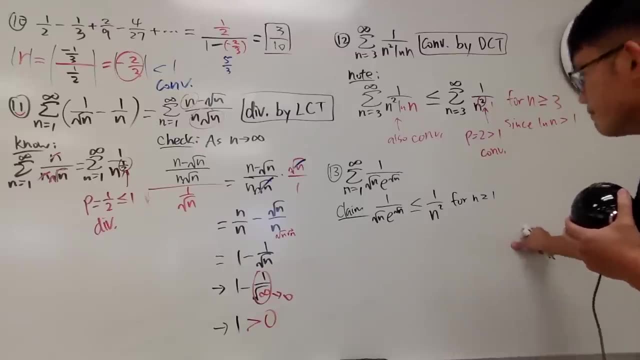 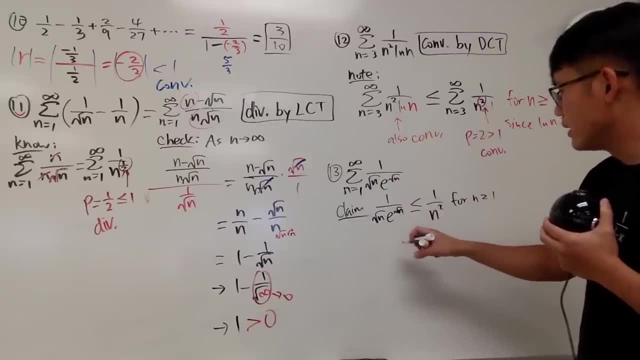 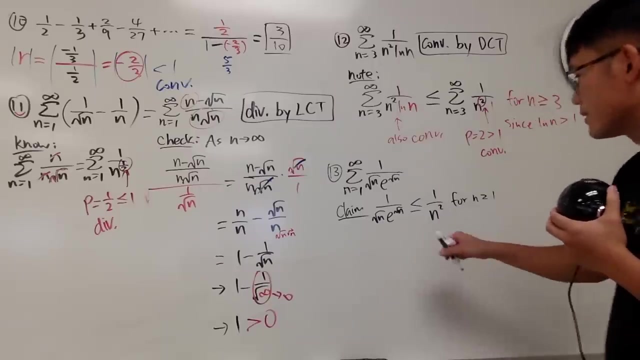 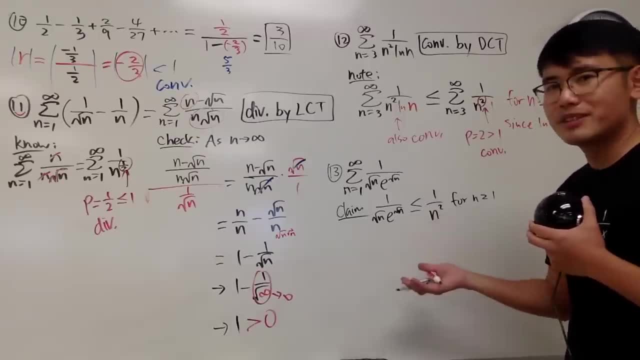 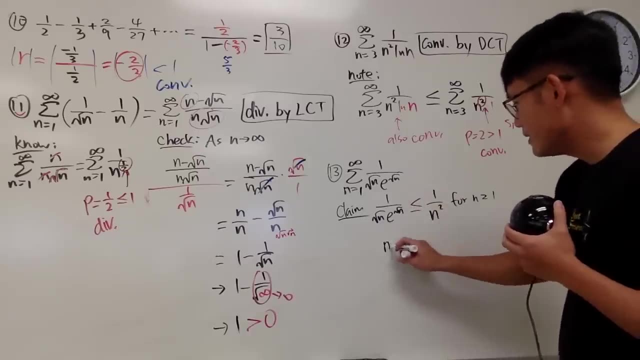 This right here is kind of like. I will do this along with the limit comparison test. Let's see, make sense, we'll see, we'll see. I will just cross multiply. we get n square which is less than or equal. 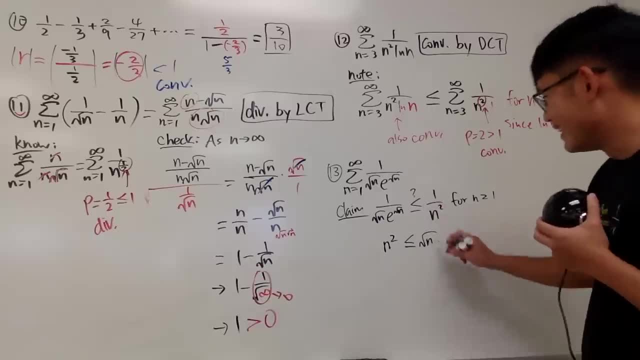 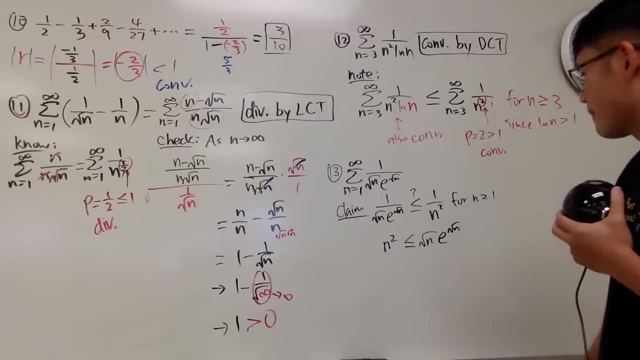 to square root of n- Oh, by the way, I don't know yet- And um e to the square root of n. right here, right, And hmm, let's see, let's see, let's see. 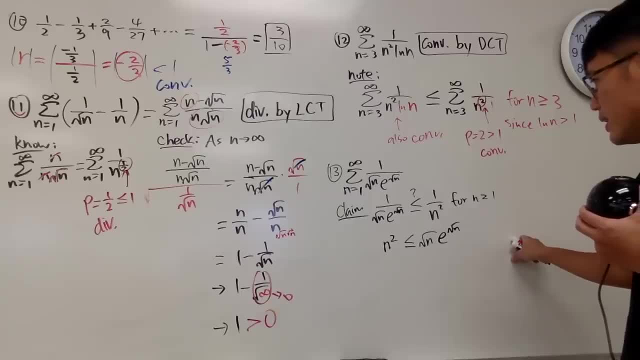 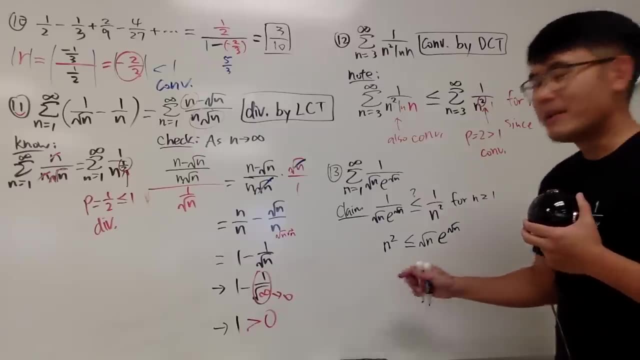 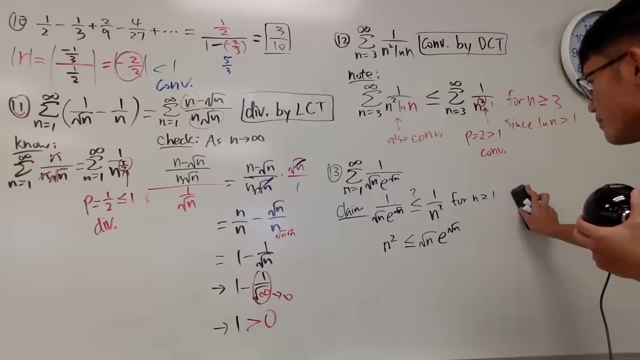 hmm, wait a second. the truth is, this is still true at some point. Okay, let's do it this way. Hm I? I can still simplify the expressions if you guys would like me to do so, I think I will just do that, why not? 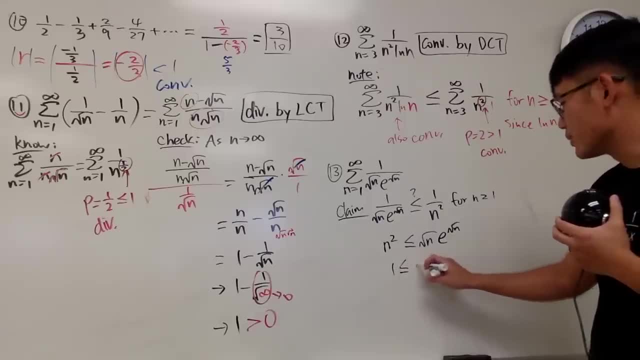 So this is 1 less than or equal to square root of n, e to the square root of n over n squared. And the idea is this is 1 less than or equal to simplify this, this is I'm saying n times n. 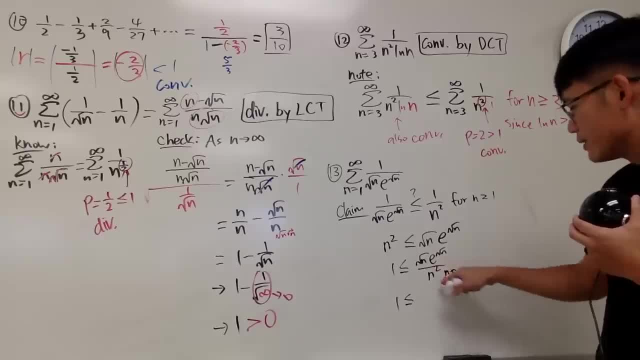 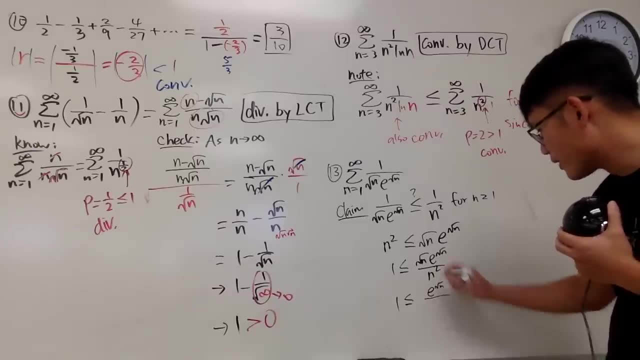 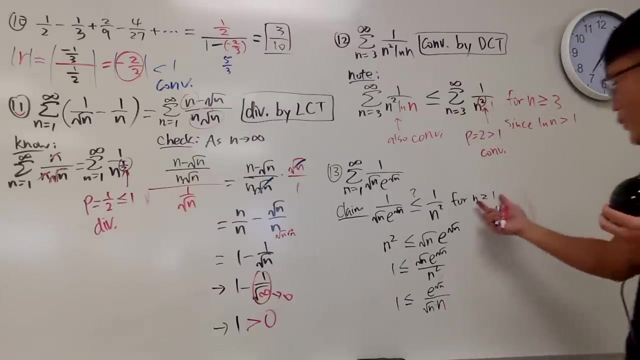 which is square root of n, square root of n times that. So you can simplify this a little bit and you end up with e to the square root of n over square root of n times. n like this right And the truth is, when n is greater or equal to 1, this right here is, of course, bigger than 1, okay. 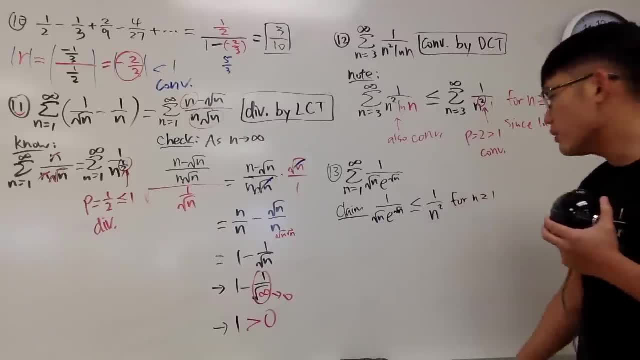 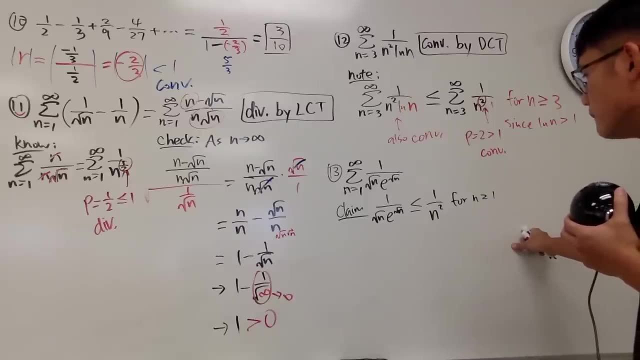 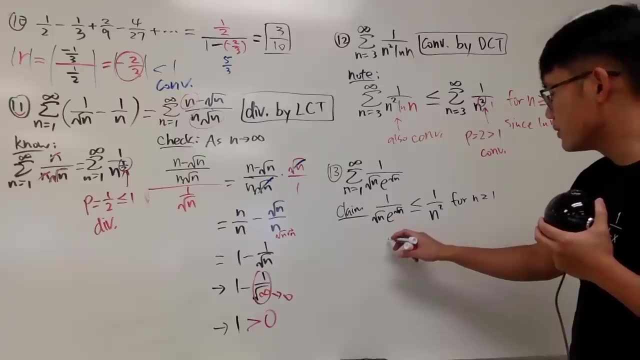 for n greater than or equal to 1.. Now let's see how can we make that happen. Well, you can just multiply, if you would like, so I will do that. Or maybe you can just do. let's see limit comparison test. 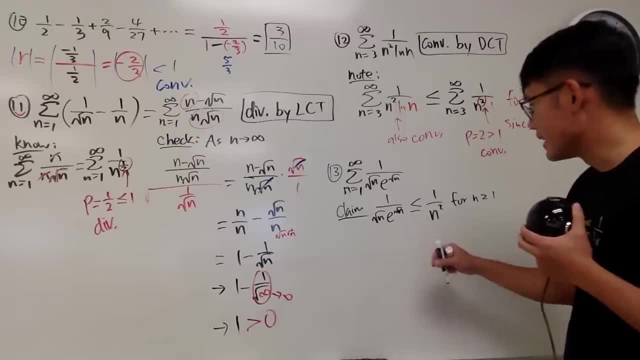 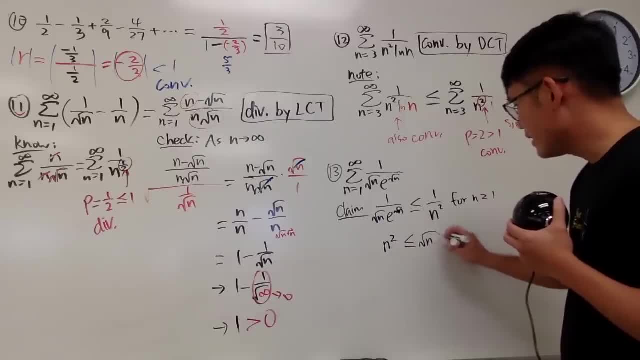 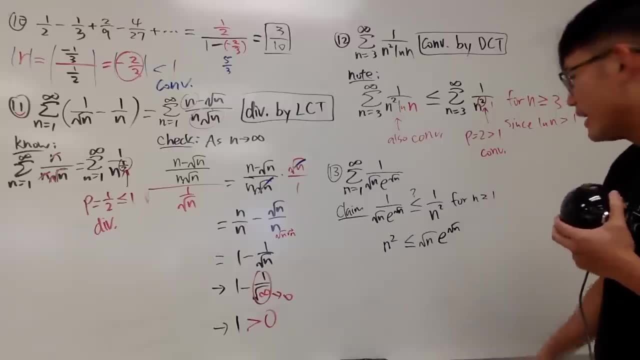 I will just cross multiply, we get n squared, which is less than or equal to square root of n- oh, by the way, I don't know yet- And e to the square root of n. right here, right, And. 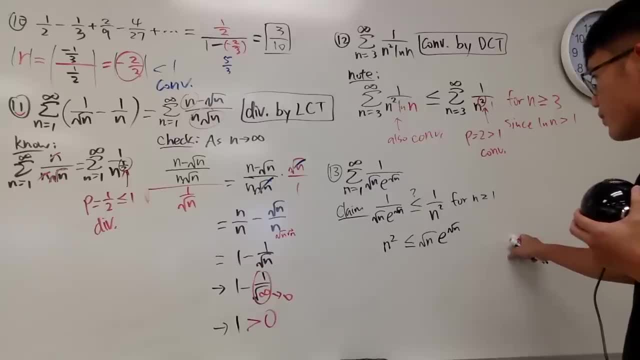 hmm, let's see, let's see, let's see. The truth is: this is still true at some point. Okay, let's do it this way. Hmm, I can still simplify the expressions if you guys would like me to do so. 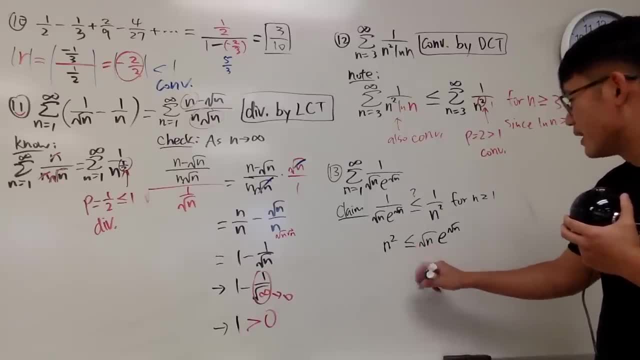 I think I will just do that, why not? So this is 1 less than or equal to square root of n, e to the square root of n over n squared, and the idea is this is 1 less than or equal to. 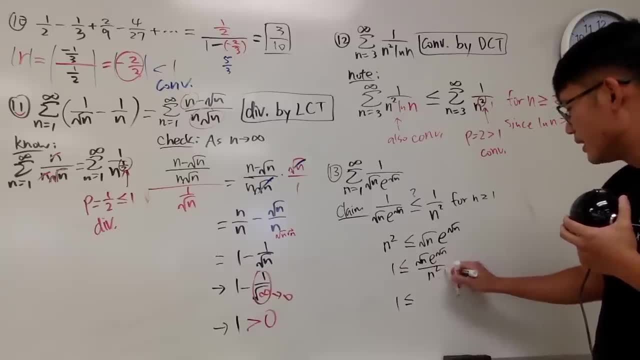 simplify this. this is like saying n times n, which is like square root of n, square root of n times that. So you can simplify this a little bit and you end up with e to the square root of n over. 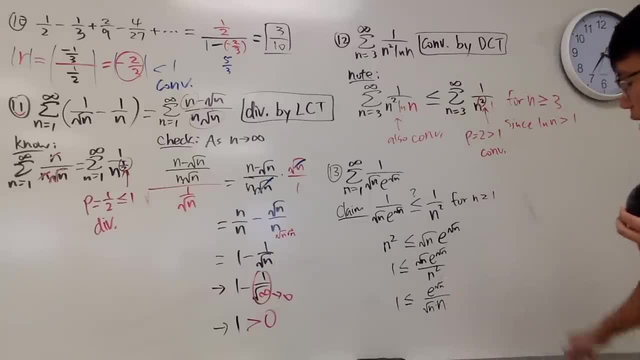 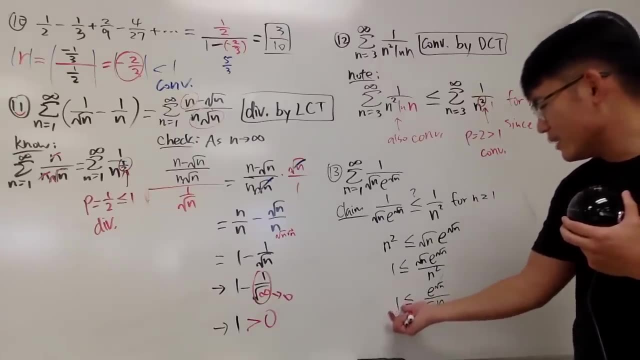 square root of n times n like this right. And the truth is, when n is greater than or equal to 1, this right here is, of course, bigger than 1, okay, So this right here you can say, is true. 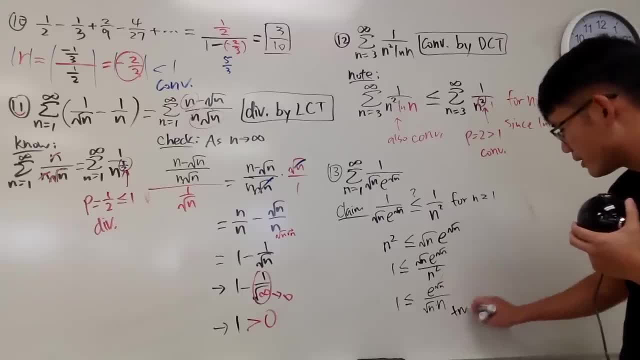 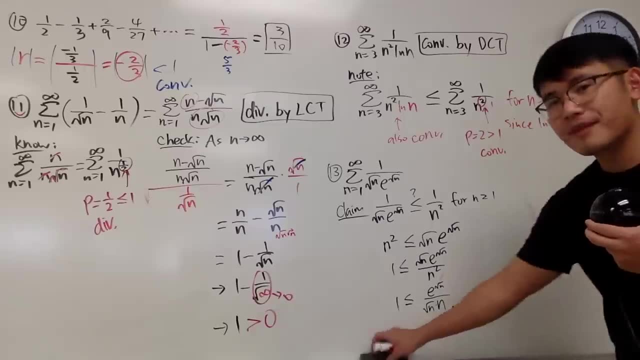 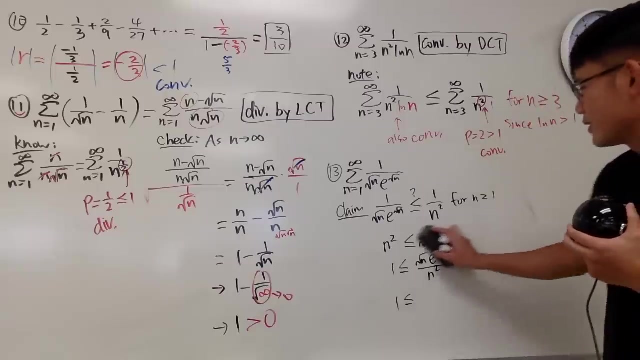 So this right here you can say is true by the list, because you have the power of that. Okay, all right, let's do this. What about this? Let's do this, Let's just do this again. All right, here's the deal. 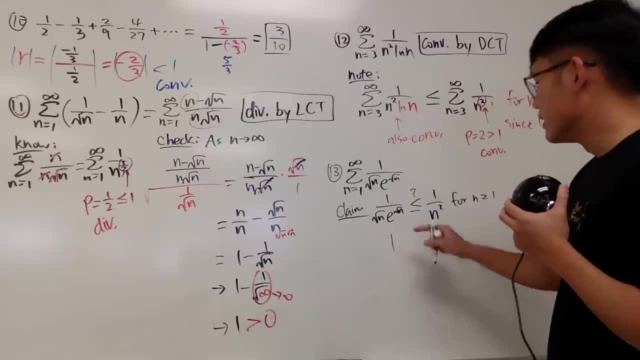 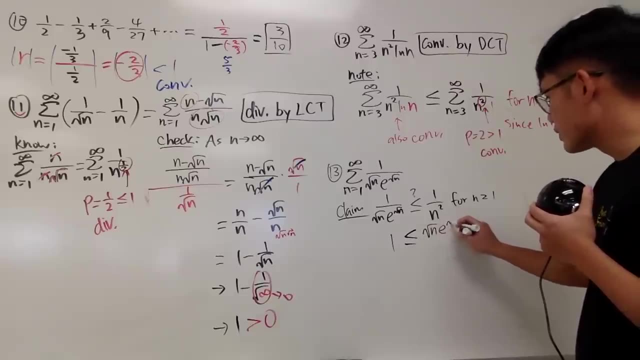 I'm going to multiply this on both sides. I'm just going to check if this right here is, we'll have the square root of n e to the square root of n over n, squared right here. right, And this right here. simplify this and that. 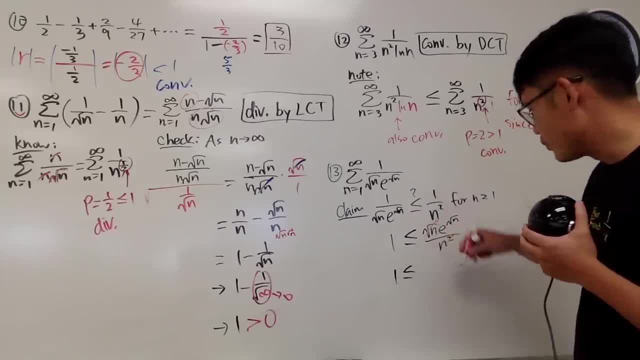 This is, I'm saying 1 half power. This is I'm saying 4 over 2.. So you can do the powers on your own. You get 3 half right here. So we have e to the square root. 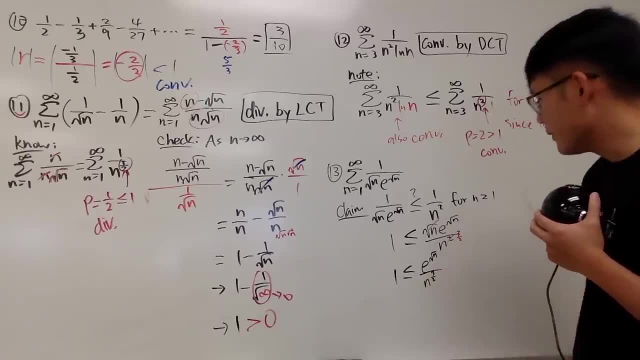 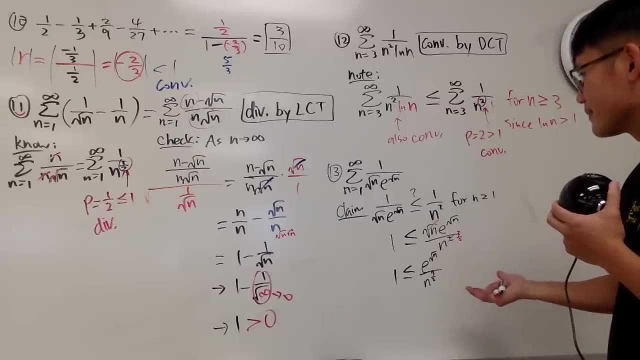 So we have square root of n over n to the 3 half power, And now I will do a small change of variable, because this right here is technically not. Oh man, I could have just done that in the beginning, That might be even better. 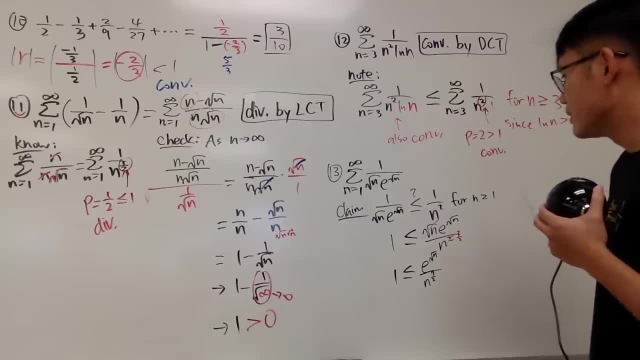 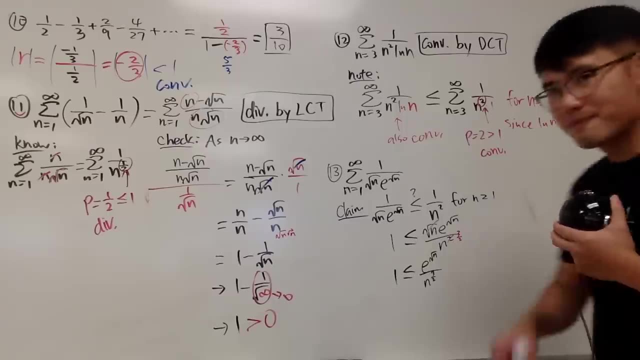 Let's see if you guys would like this or not. Let's see if I do the square root of n and change the square root of n to, let's say, I'll do that Much better. Okay, So you guys can see, I'm really just working this out. 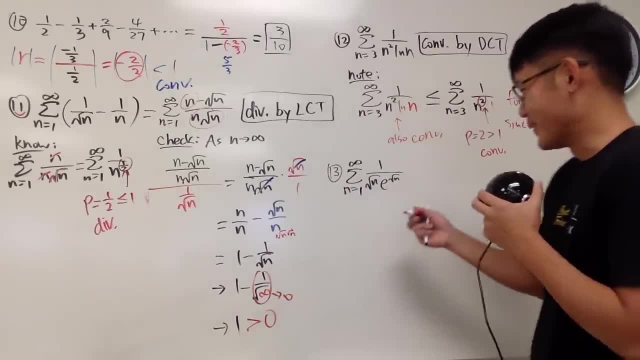 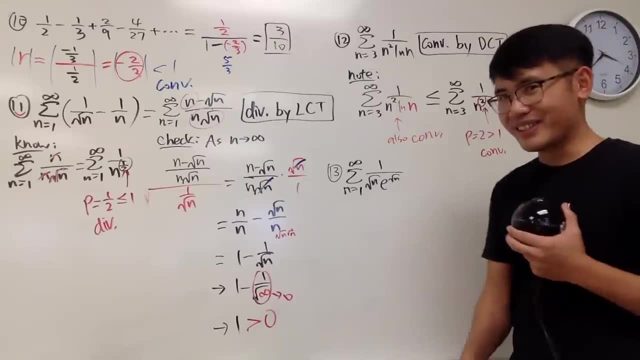 I just prepared the questions I want to test out, but I'm really working this out along the way. So here we'll do a substitution just like an integral, but hopefully you guys don't get too excited. Anyway, I will just let. do you guys want to use u? 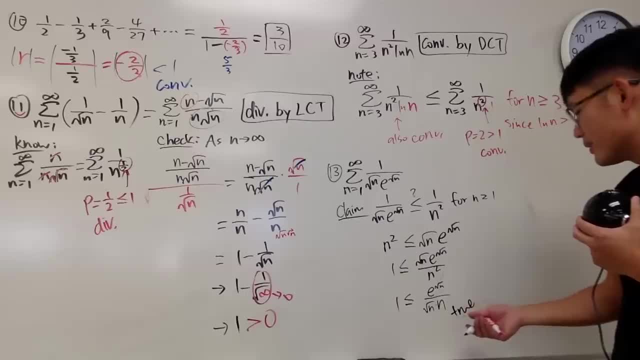 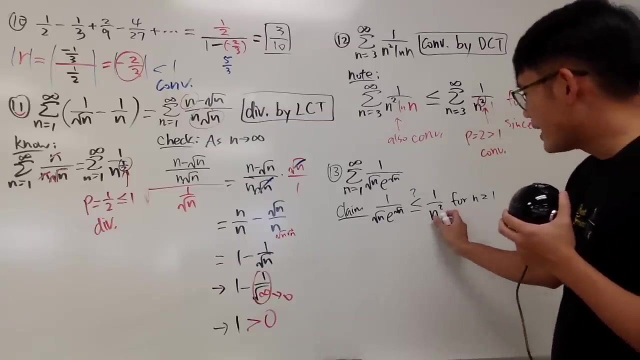 by the list, because you have the power of that. Okay, Alright, let's do this. What about this? Let's do this. Let's do this again. Alright, here's the deal. I'm going to multiply this on both sides. 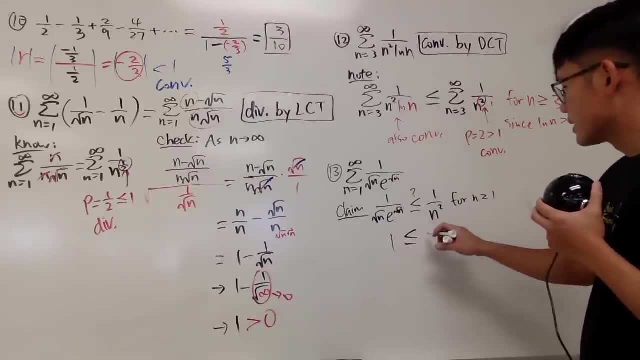 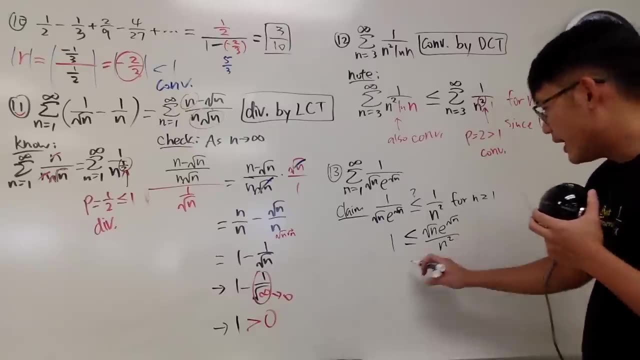 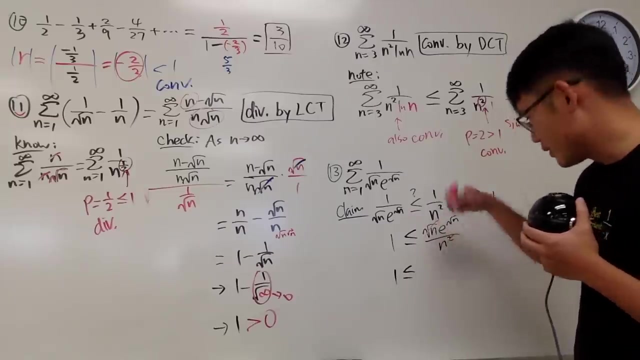 I'm just going to check if this right here is. we have the square root of n e to the square root of n over n, squared right here. right, And this right here, simplify this, and that this is like saying 1 half power. 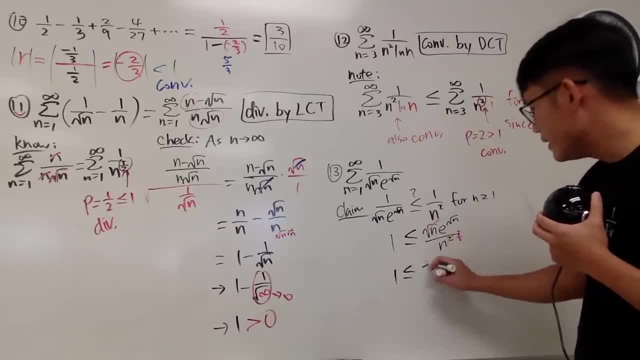 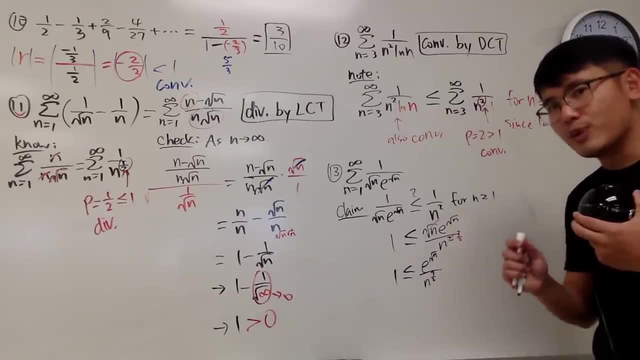 this is like saying 4 over 2, so you can do the powers on your own. you get 3 half right here. So n to the 3 half power. and now I will do a small change of variable, because 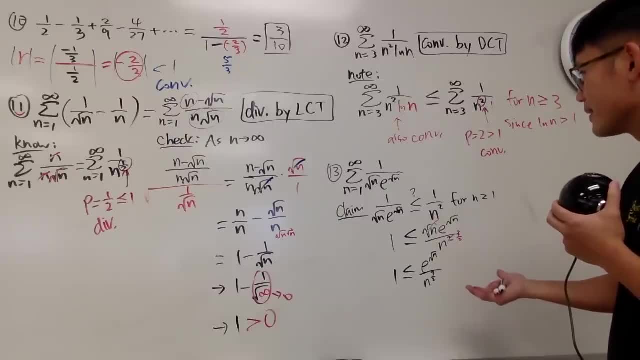 this right here is technically not. Oh man, I could have just done that in the beginning. That might be even better. Let's see if you guys would like this or not. Let's see if I do the square root of n and change the square root of n to: 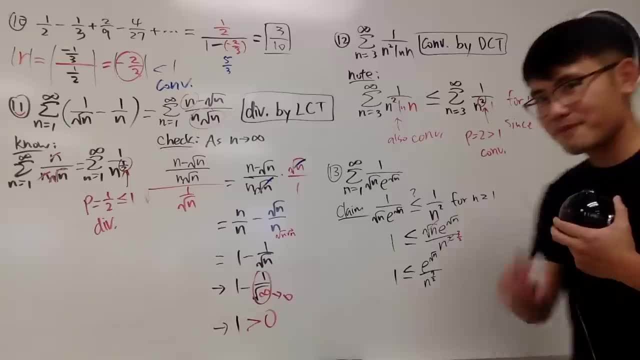 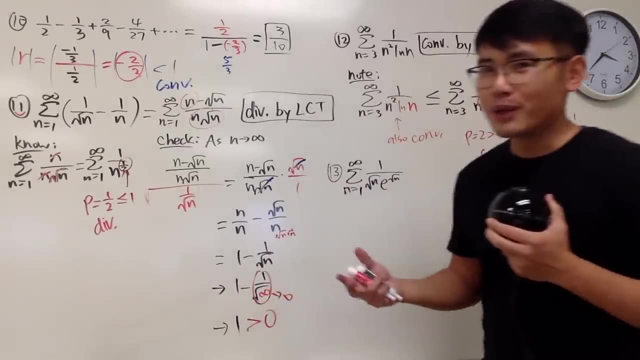 let's say I will do that Much better, okay? So you guys can see I'm really just working this out. I just prepared the questions I want to test out, but I'm really working this out along the way. So here we will do a. 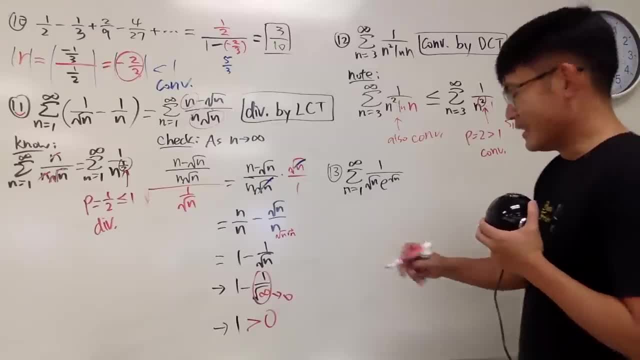 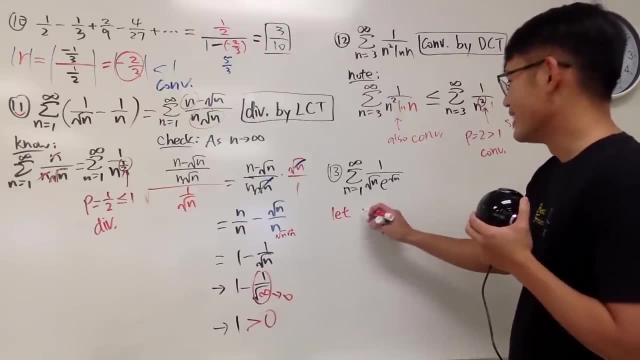 substitution, just like an integral, but hopefully you guys don't get too excited. Anyway, I will just let. do you guys want to use u? Oh, no, no, up to you. I will use m because technically this right here should be whole numbers. 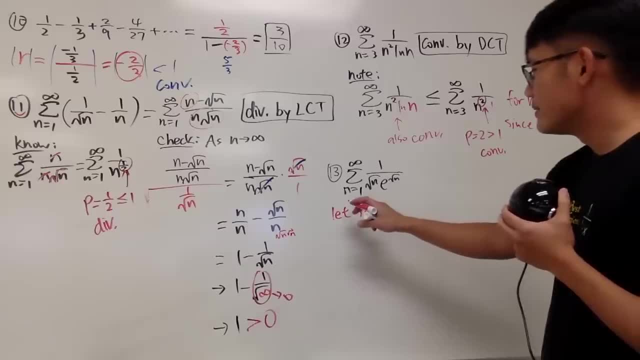 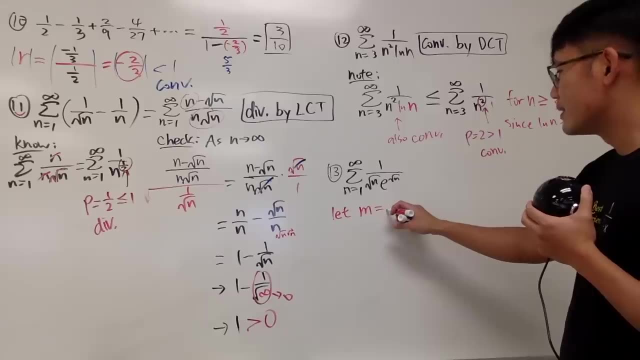 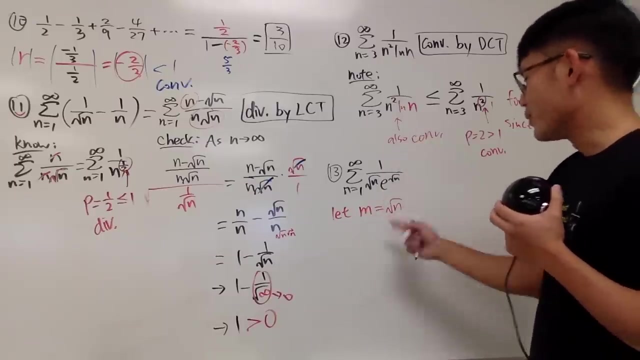 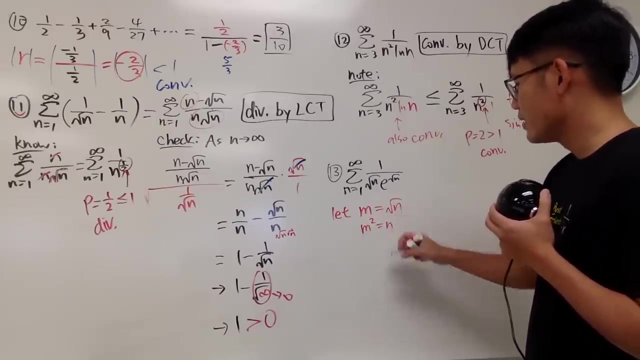 So I will let m to be square root of n. Okay, Whatever It should be, okay, Yeah. And if you and you get m squared is equal to n Okay. this right here, it's that's. that's just through the integrals. 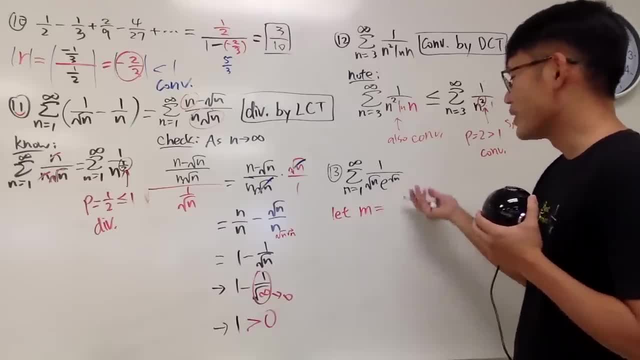 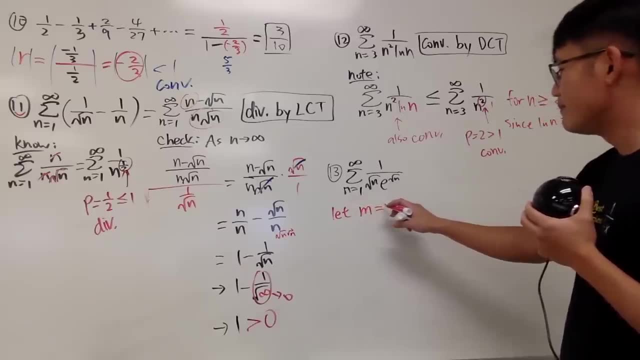 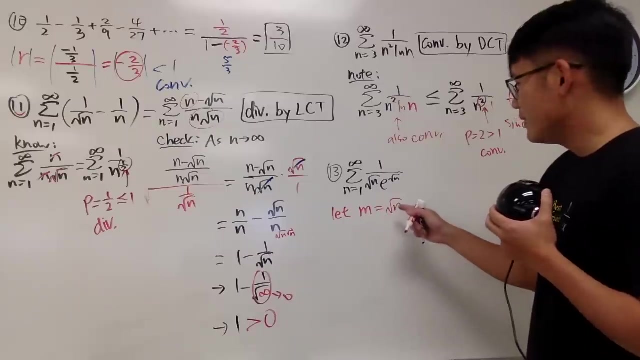 Oh, no, up to you, I'll use m because technically this right here should be whole numbers. So I will let m to be square root of n. Okay, Whatever, It should be okay, Yeah. And if you. 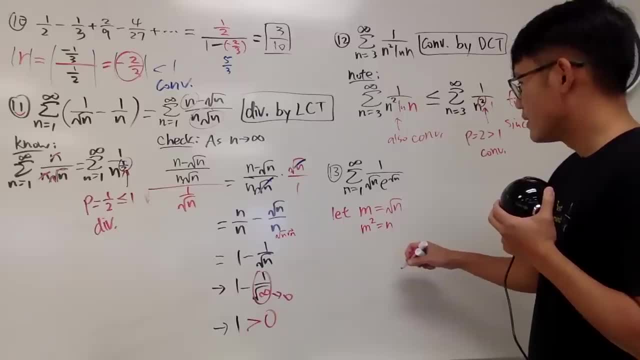 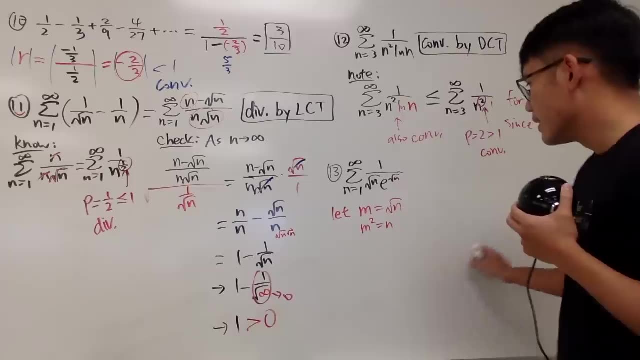 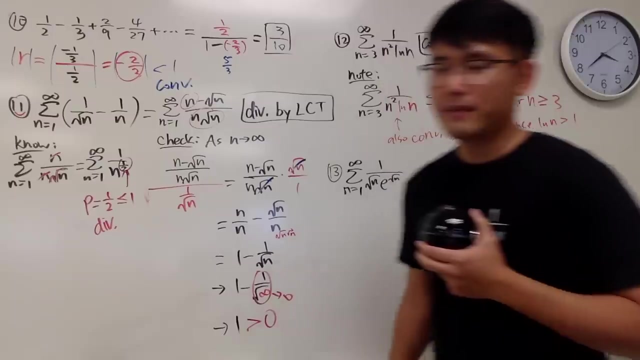 And you get m squared is equal to n. Okay, this right here, it's that's. that's just two of the integrals. Okay, I'm going to just put question number 13 at test span 1, 1, 4.. 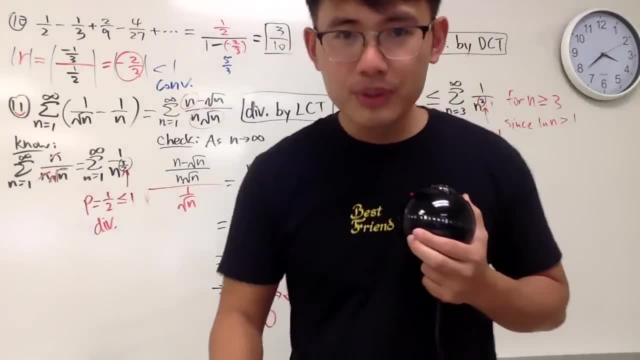 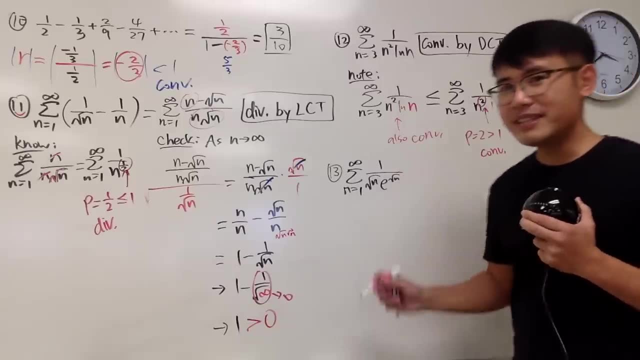 Okay, I'm going to just put question number 13 at test band 114.. Okay, that will be my stretch. Okay, so let's take a look at this series as n goes from 1 to infinity of 1, over square root of n, e to the nth power. 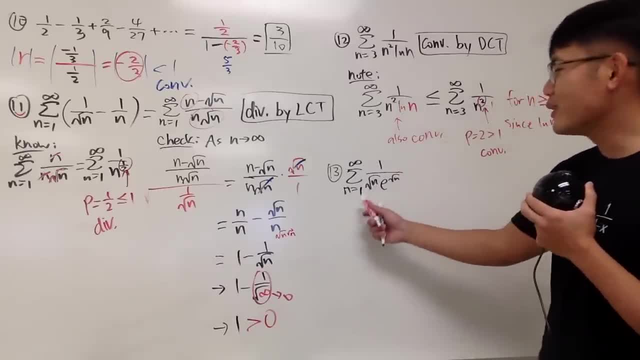 Okay, that will be my stretch. Okay, so let's take a look at this series as n goes from 1 to infinity of 1 over square root of n, e to the nth power, right here And now. here is the deal. 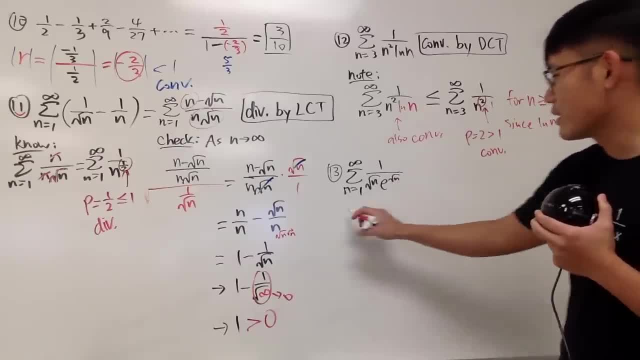 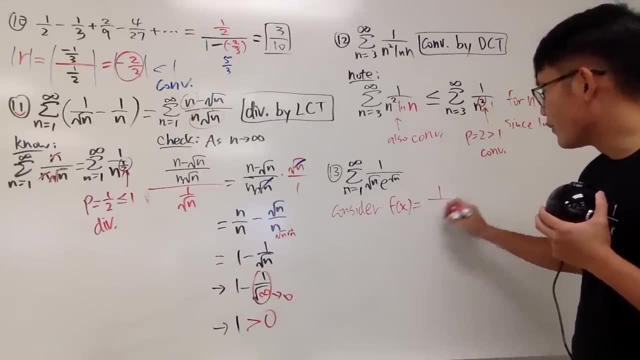 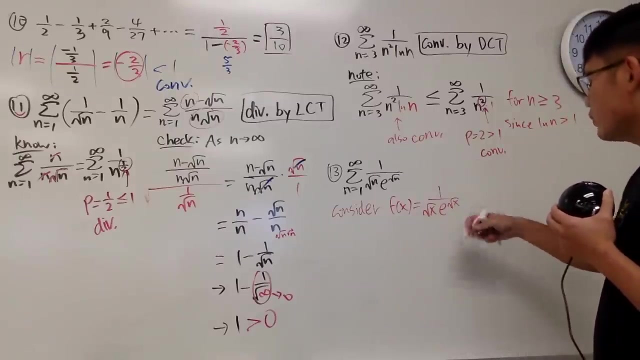 We can actually use the integral test for this, because we can. we can go ahead and consider: well, consider: f of x is equal to 1 over square root of x, e to the square root of x, power like this. And, of course, when you have this: 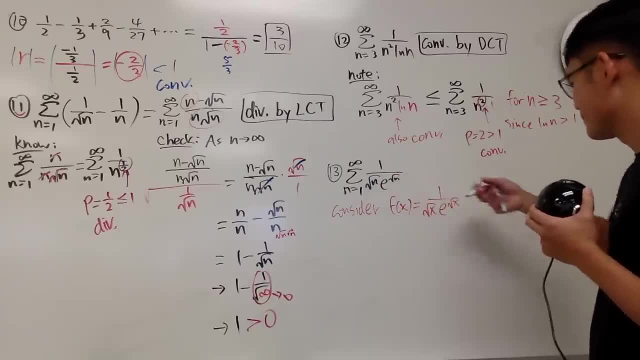 just go ahead and put down the, the graph, And seriously, the graph will almost always look like this, right, Something like that, And it's going to be increasing, so it's going to be decreasing and then positive over that. 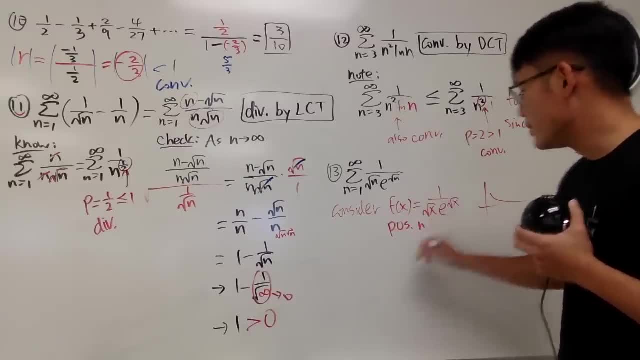 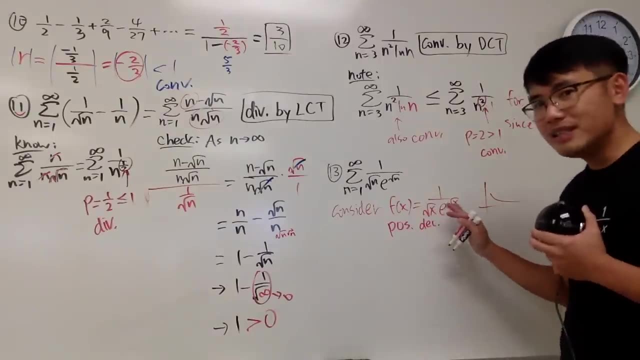 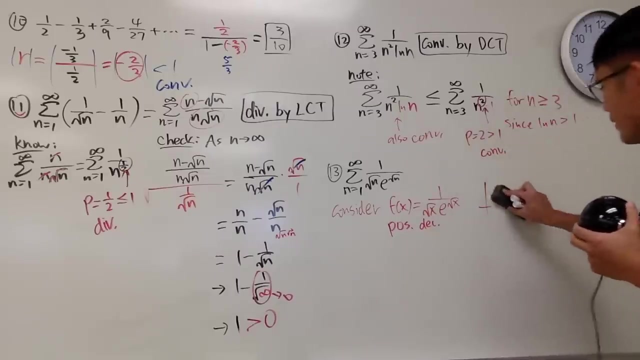 So just go ahead and say positive and decreasing and all the good things that will be needed, Even though, to be honest, even though it may be like a little up, a little bit, but eventually it will be decreasing. So I don't know, but this is the deal, right. 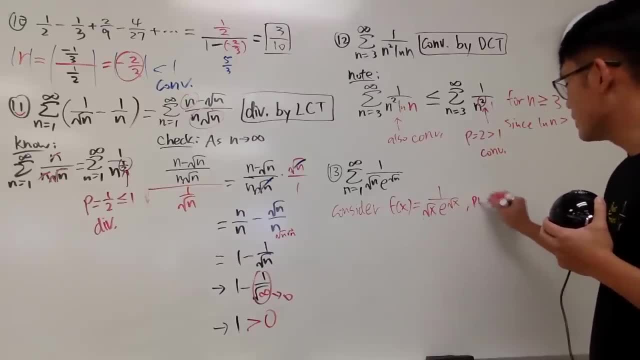 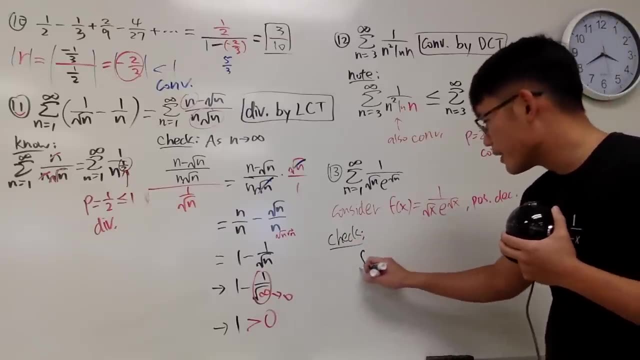 So I'll just put this down right here like positive decreasing. And now we will just check the integral. check the improper integral of 1, from 1 to infinity of 1, over square root of x, e to the square root of x, dx. 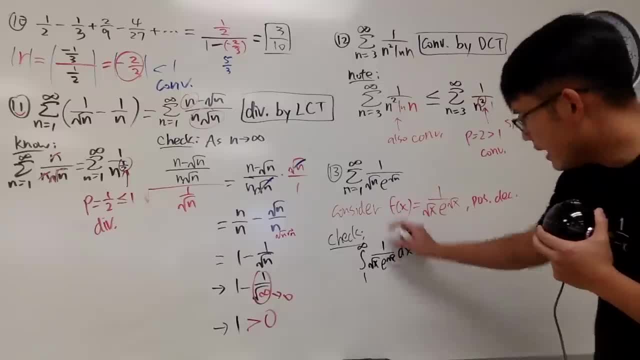 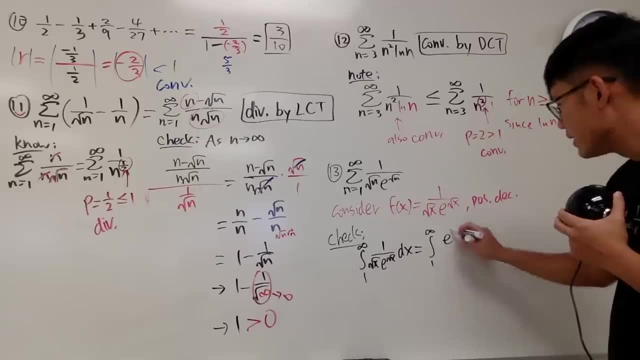 Hmm, how can we do this? Put this up a little bit and then just do a u-sub So we see this right. here is actually the integral of 1 to infinity e to the negative square root of x over square root of x dx. 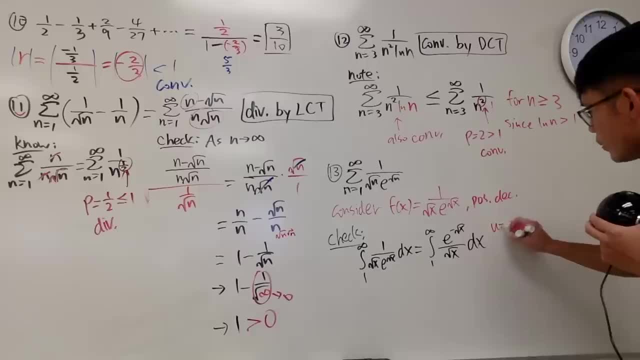 And I'll do a u-sub right here real quick for you guys. I will let u equal to negative square root of x and dx. u will be negative 1 over 2 square root of x- dx And if you would like, you can just get a dx by itself. 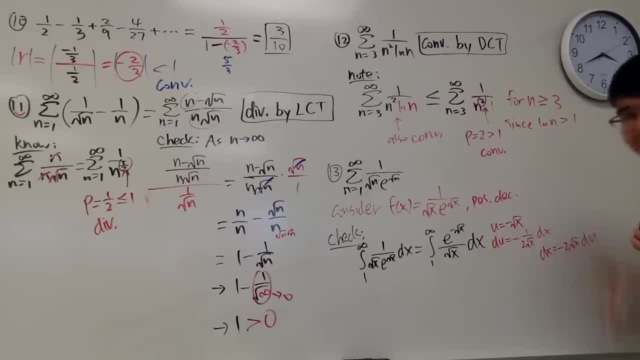 and we get negative 2. square root of x. du like this: Put this back here and don't forget to take this to the u-world. So x go from 1 to infinity. And here we have the integral u will go to. let's see: put in 1, we get negative 1.. 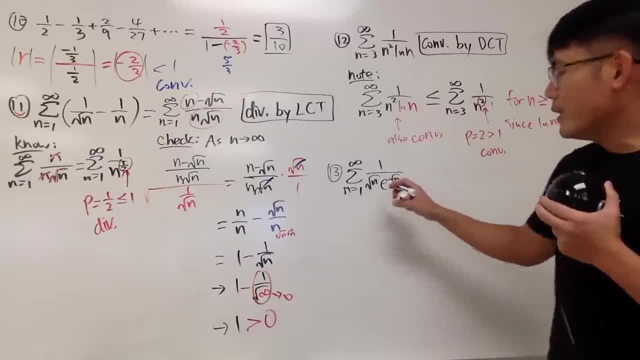 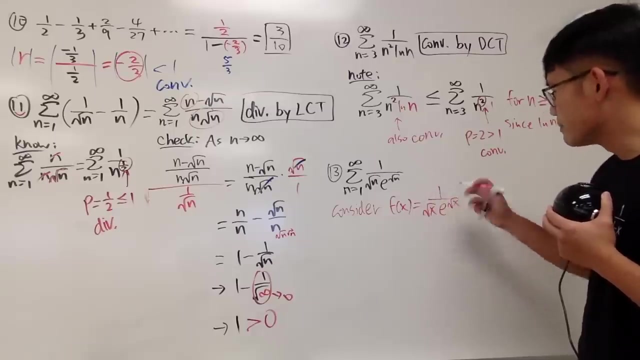 right here. And now. here is the deal: We can actually use the integral test for this, because we can go ahead and consider: well, consider: f of x is equal to 1 over square root of x. e to the square root of x power. 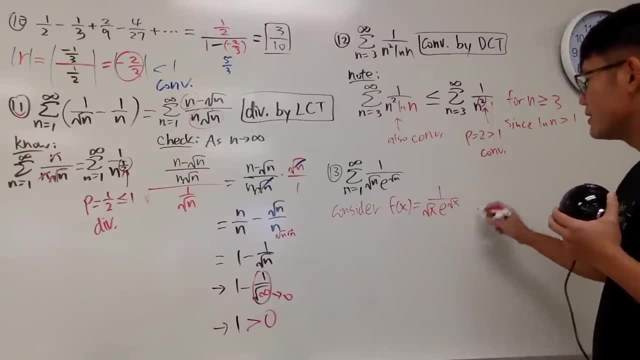 like this And, of course, when you have this, just go ahead and put down the the graph, And seriously, the graph will almost always look like this, Right, Something like that, And it's going to be increasing, so it's. 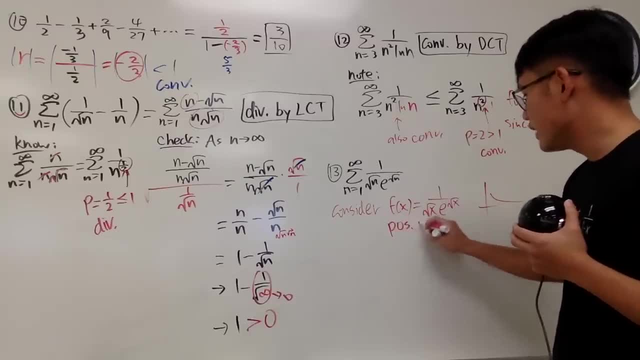 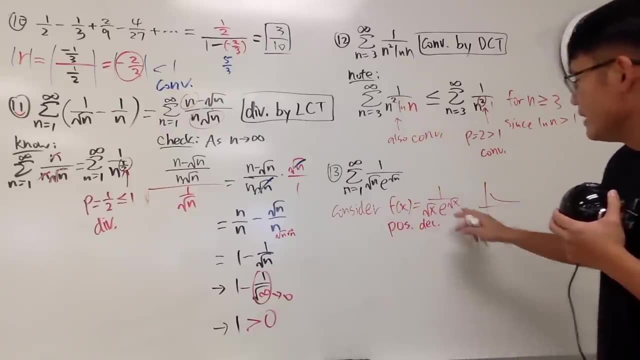 going to be decreasing and then passing over that. so just go ahead and say positive and decreasing and all the good things that will be needed, Even though, to be honest, even though it may be like a little up, a little bit, but eventually it will be decreasing. 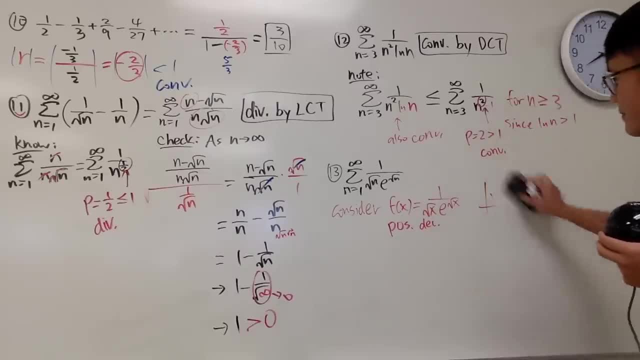 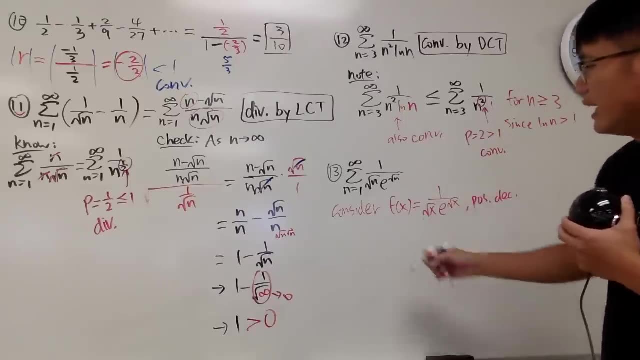 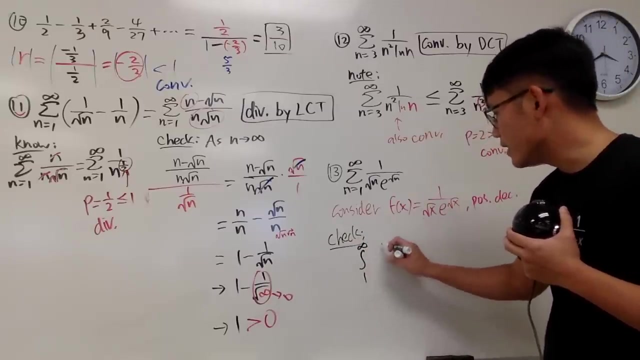 So I don't know, But this is the deal, right. So I'll just put this down right here like positive decreasing. and now we will just check the integral, check the improper integral of from one to infinity of one. 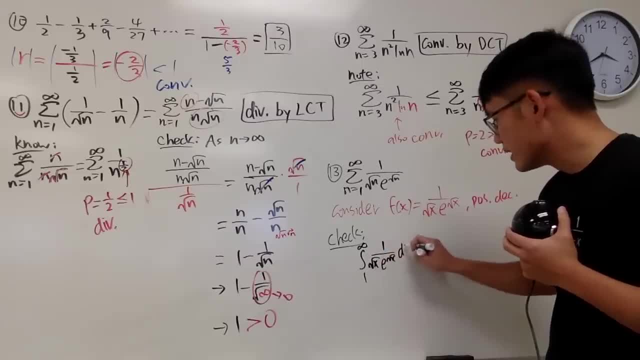 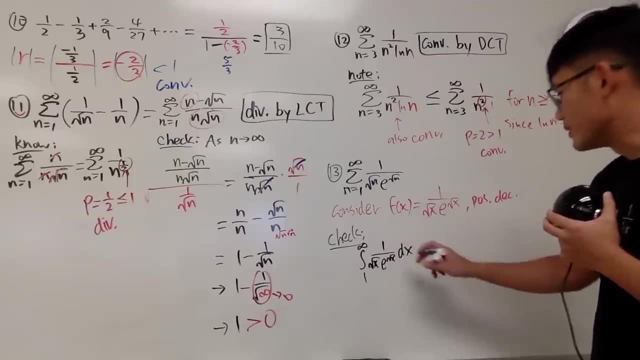 over square root of x e to the square root of x- dx. Hmm, how can we do this? Put this up a little bit and then just do a u-sub So we see this right. here is actually the integral of one to infinity. 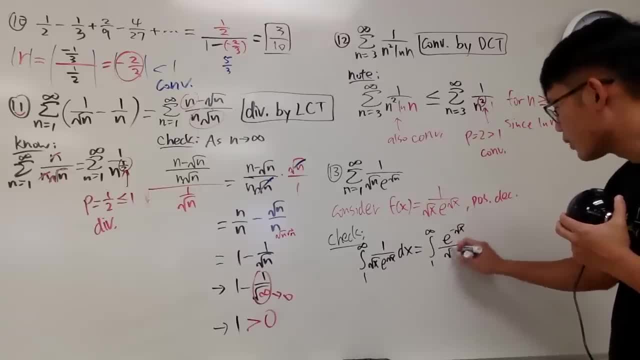 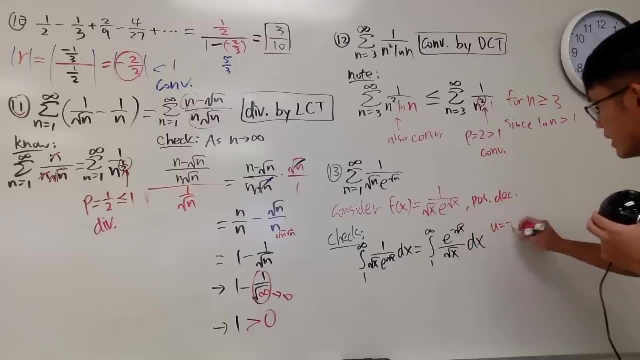 e to the negative square root of x over square root of x dx. And I'll do a u-sub right here real quick for you guys. I will let u equal to negative square root of x and du will be negative one over two square root of x. 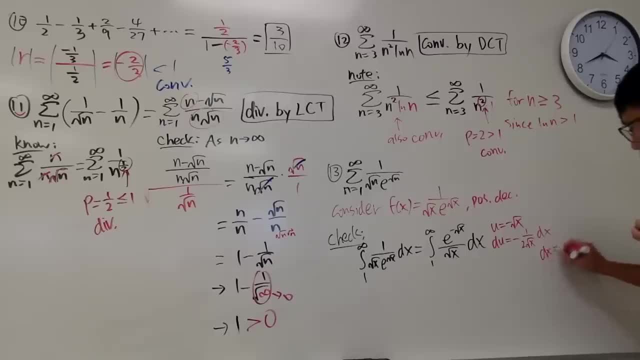 dx And if you would like, you can just get a dx by itself and we get negative two square root of x. du like this. Put this back here and don't forget to take this to the u-world. So x go from one to infinity. 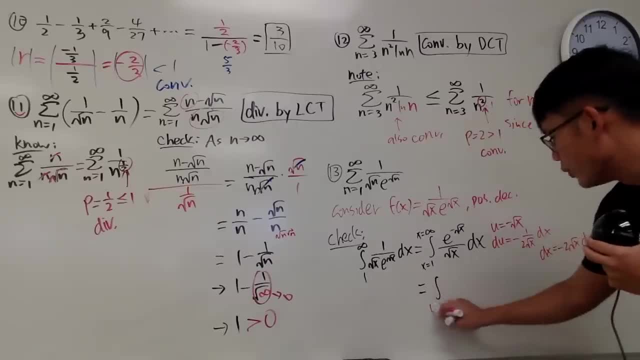 and here we have the integral U will go to. let's see: put in one, we get negative one. put in infinity- square root of infinity is infinity, then that's a negative version. So we take infinity right here and we have e. 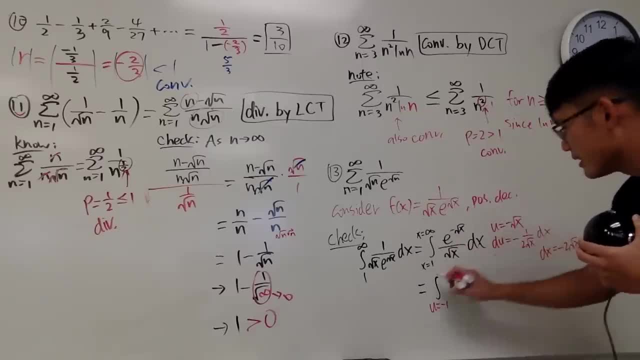 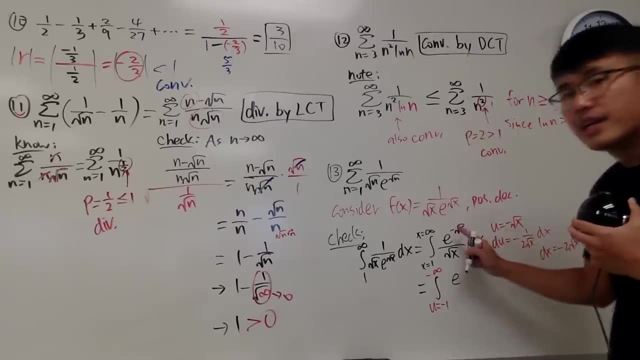 Put infinity. square root of infinity is infinity and that's a negative version. so negative infinity right here. And we have e on the top, we have u, because I take the negative square root of x to be the u over this right here is just square root of x. 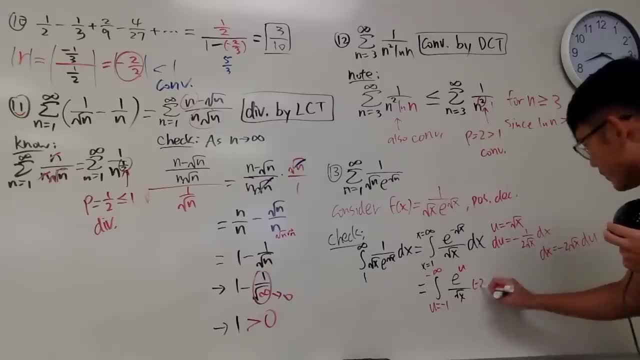 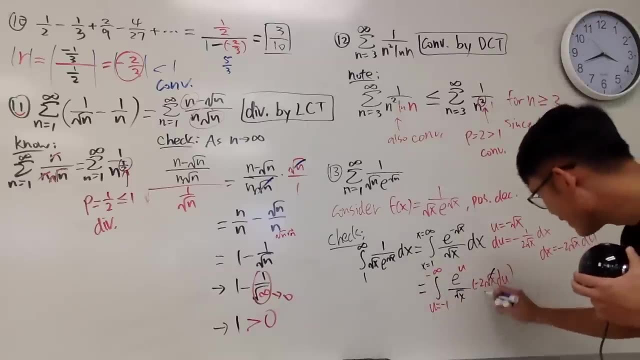 Let me put that down. And dx is this, which is negative 2 square root of x. du like that. And of course we can see that this and that cancel And all in all we are going to do two things. 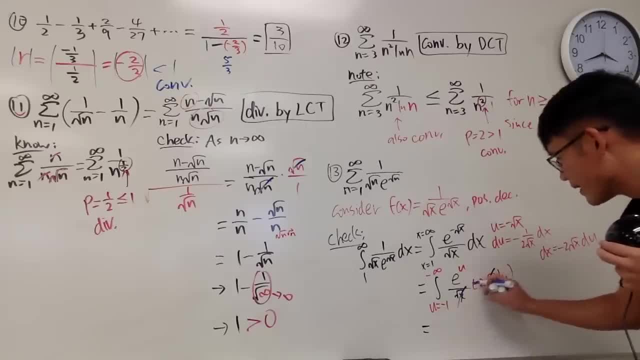 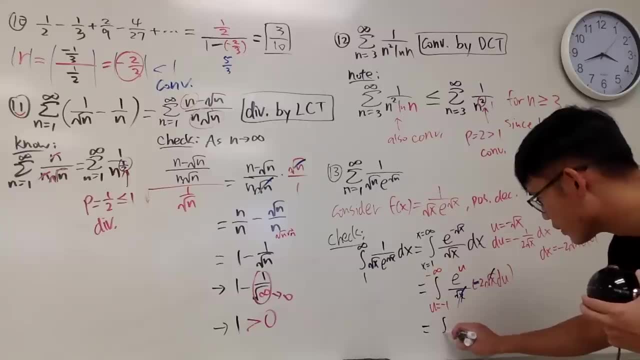 First, You see that we have the negative right here. This negative, we can switch the limits of integration to water, right, So we get positive, going from negative infinity to negative 1, and then we have 2 right here, all the way in the front. 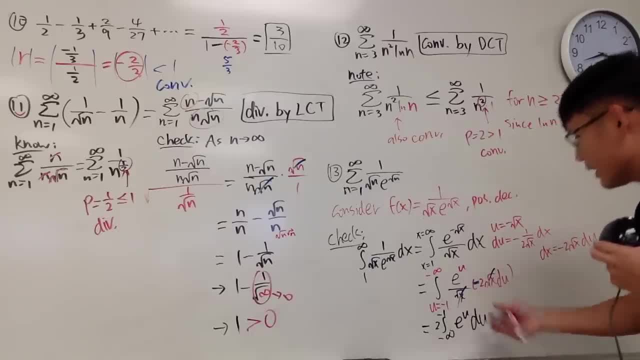 and then we have e to the? u's power. du like this, Alright, And of course you can just integrate this real quick in the u-world and we finish that in the u-world. We have 2, and then the integral of that is just e to the? u. 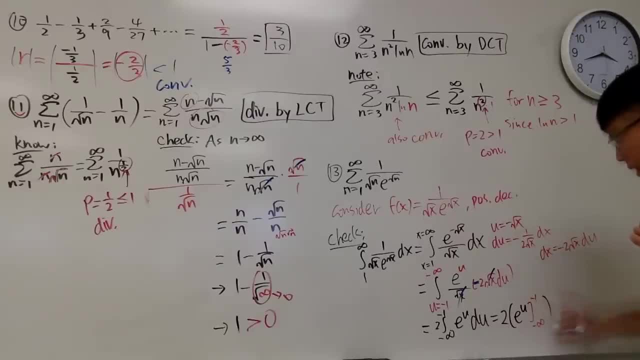 and we go from negative infinity to negative 1, like this: And if you put negative 1, and you put infinity, negative infinity, we will get this 2 times e to the negative 1, minus e to the negative infinity, like that. 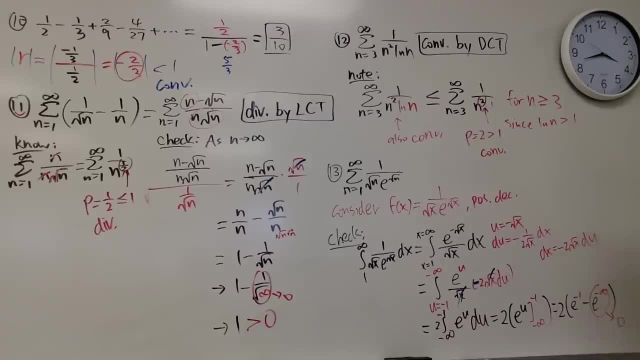 And, of course, this right here goes to 0. This right here is finite, which is actually just 2 over e. right here, right, But don't be too excited. Don't be too excited about this number. All in all, we just have to know that this right here is finite. 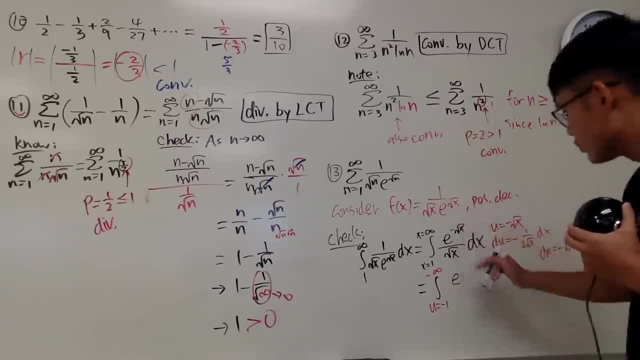 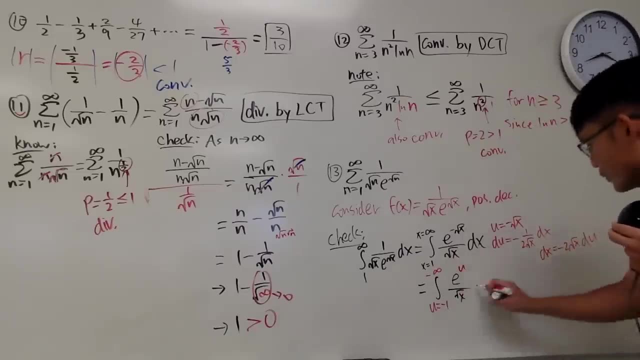 on the top we have u, because I take the negative square root of x to be the u over. this right here is just square root of x, Let me put that down. And dx is this, which is negative two square root of x. du like that And. 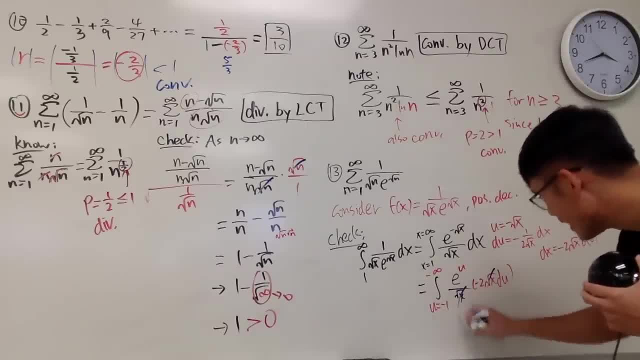 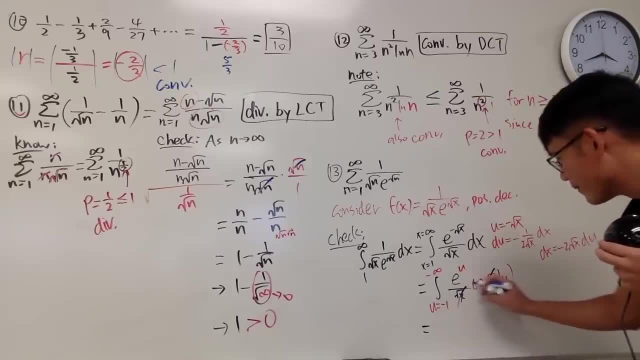 of course we can see that this and that cancel And all in all we are going to do two things. First, you see that we have the negative right here, This negative. we can switch the limits of integration to water, right. 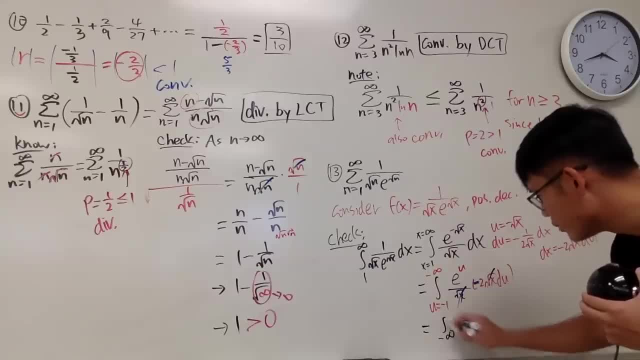 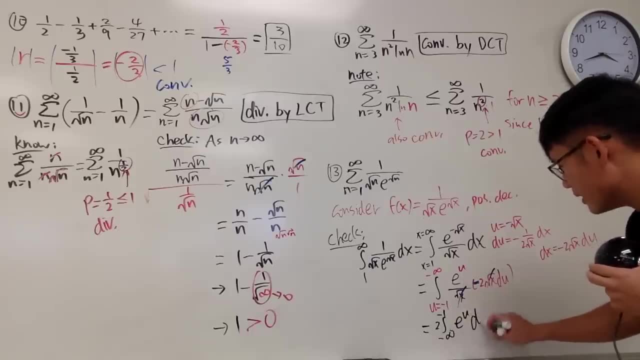 So we get positive, going from negative infinity to negative one, and then we have the two right here all the way in the front, and then we have e to the? u's power. du like this, Alright, And of course you can just integrate this real quick in the? u-world and we 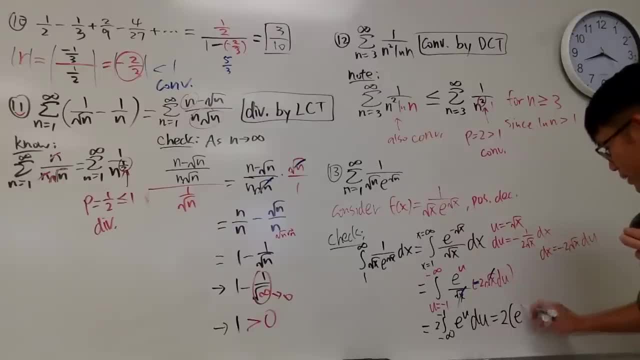 finish that in the u-world We have two and then the integral of that is just e to the u and we go from negative infinity to negative one, Like this, And if you put negative one and you put infinity, negative infinity, we will get. 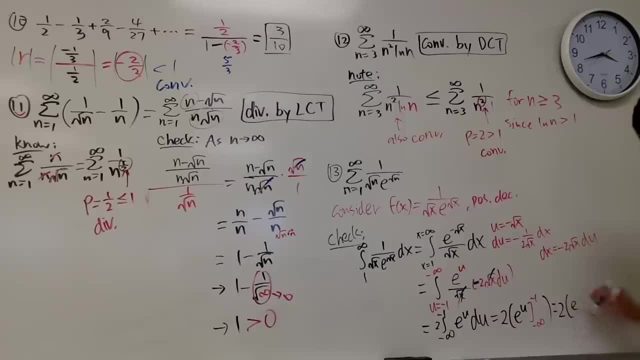 this Two times e to the negative one minus e to the negative, infinity, like that. And of course this right here goes to zero, This right here is finite, which is actually just two over e. right here, right, But don't be too excited about this number. 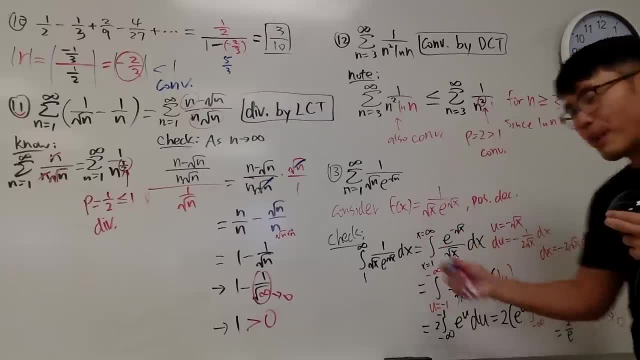 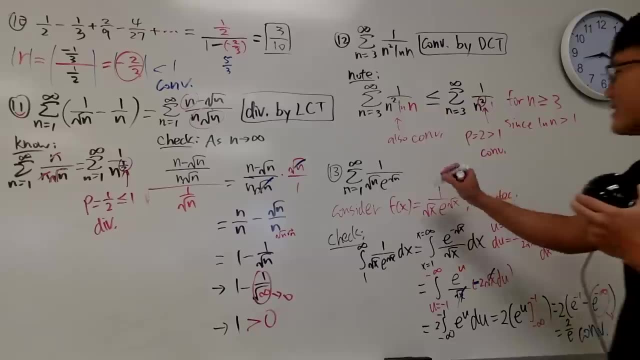 All in all, we just have to know that this right here is finite. in another word, This improper integral converges. Let me just put down this improper integral converges So we can come back here and say: this infinite series also converges by. 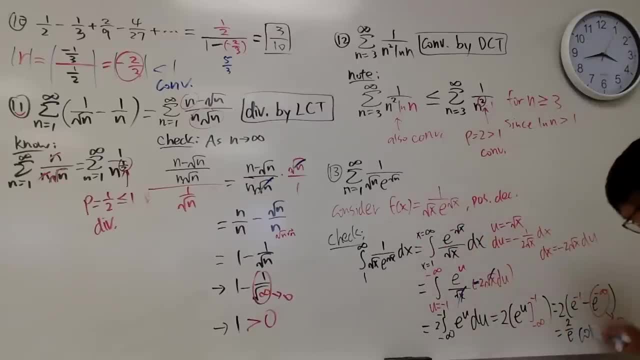 In another word, this improper integral converges. Alright, Let me just put down this improper integral converges, So we can come back here and say this infinite series also converges by integral test. i t Alright. So that's pretty much it. 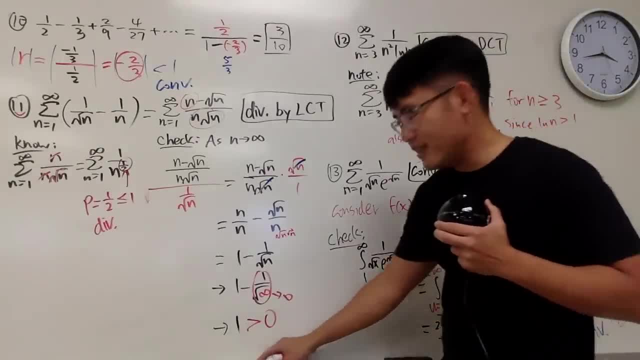 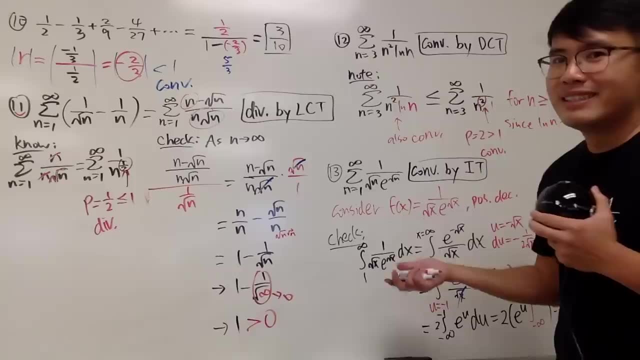 And I just didn't feel comfortable by writing: m is equal to square root of n, and take the substitution for that, because when I put down the sum that should be like whole numbers, right? So if you have square root of phi, 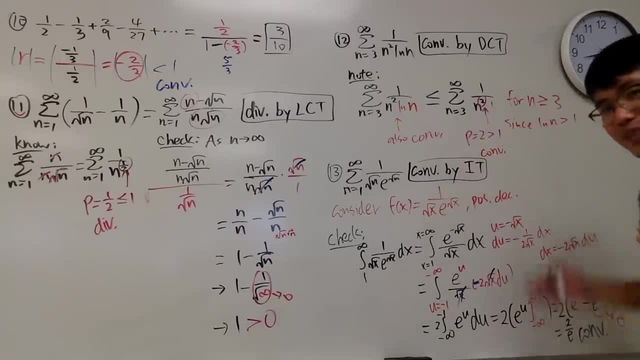 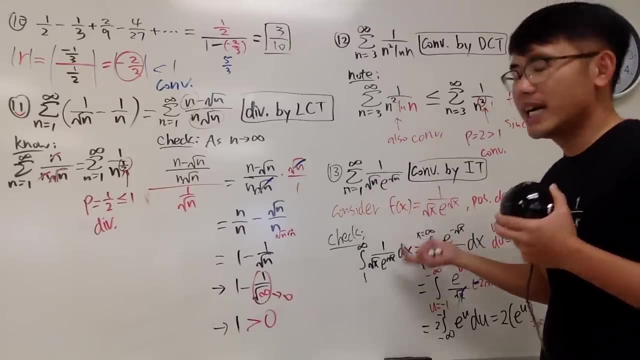 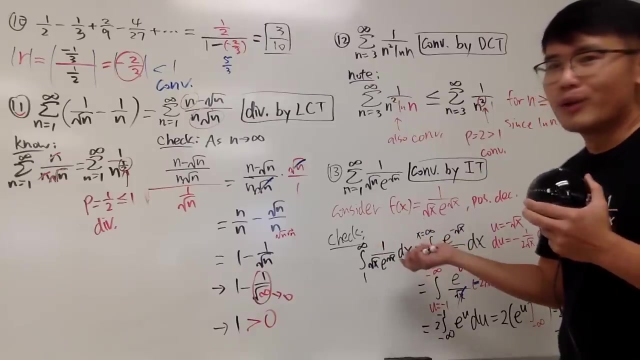 integral test: i t Alright, So that's pretty much it, And I just didn't feel comfortable by writing: m is equal to square root of n, and take the substitution for that, because when I put down the sum that should be like whole numbers. 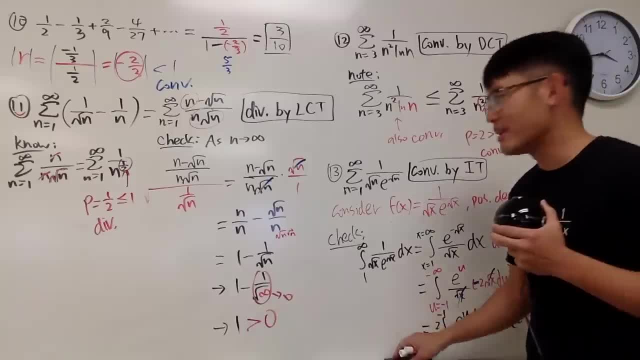 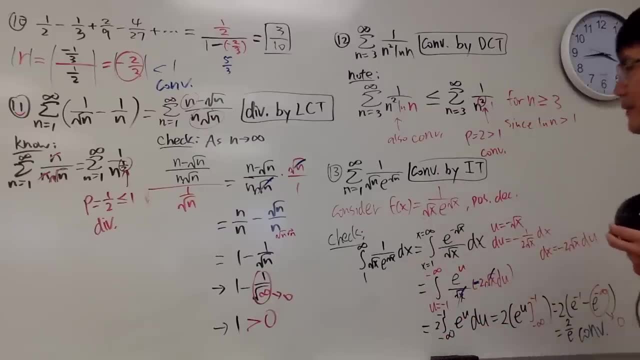 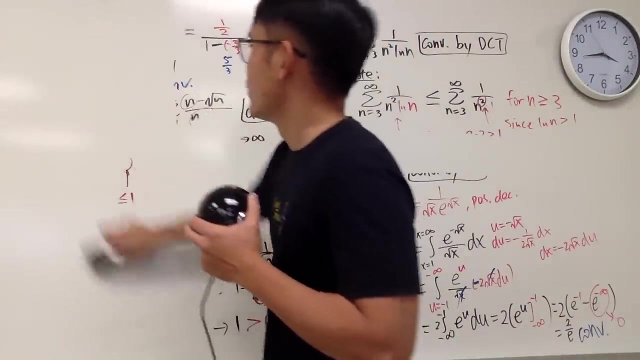 right. So if you have square root of phi, that doesn't really make that much sense. But anyway, that's my thought. but yeah, So take a look, Alright. Alright, so number 13.. That was number 13,, and then we have a lot more to go. 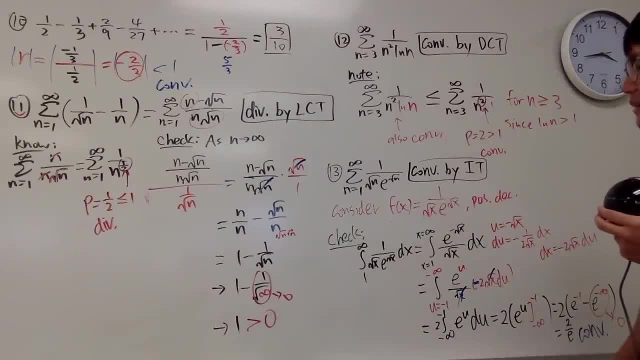 that doesn't really make that much sense. But anyway, that's my thought. but yeah, So take a look right. Alright, so number 13. That was number 13, and then we have a lot more to go. 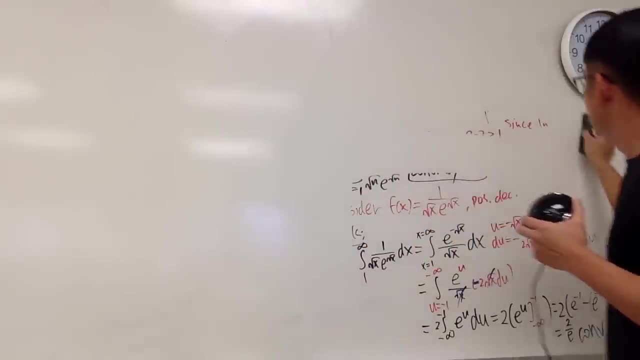 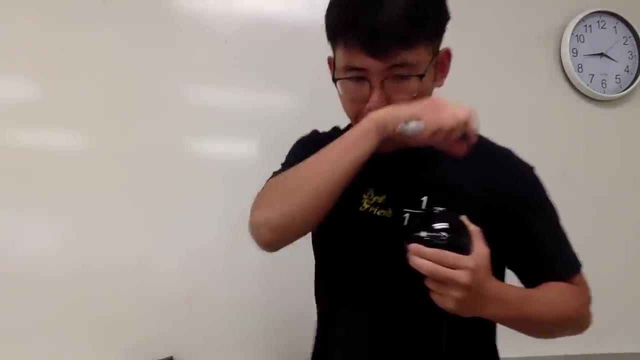 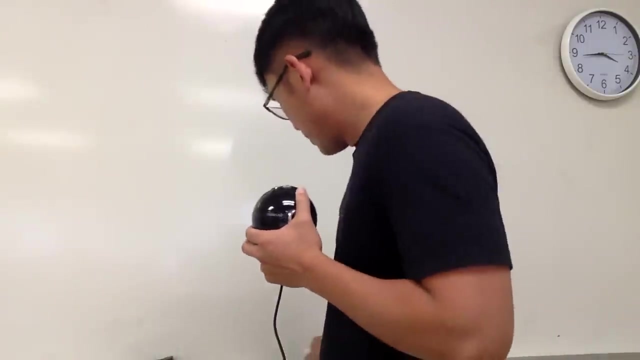 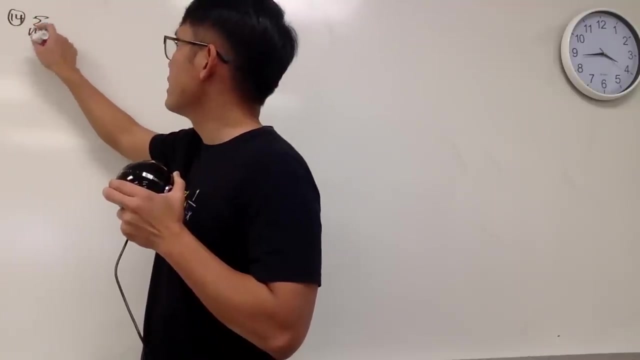 Okay, number 14, top one as well, Let's see. But finally we can do something slightly more computational for the people who like the computational stuff. Number 14. We are looking at the sum as n goes from 1 to infinity. 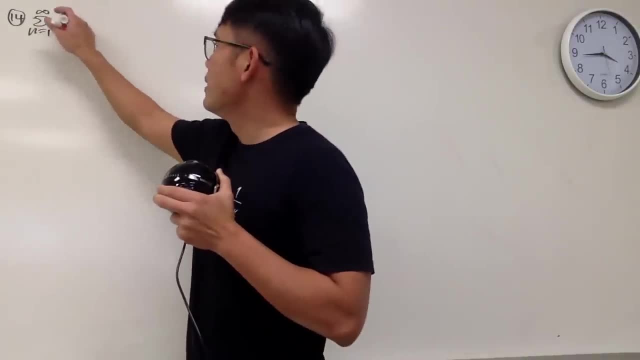 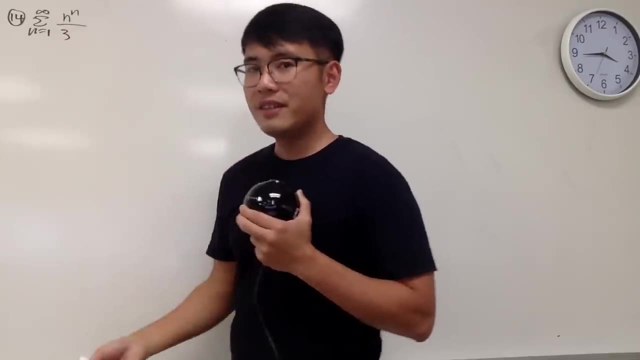 and we have n to the nth power. yes, oh my god, this is n to the nth power. It's like again like the big boss, like Thanos, right, But on the bottom we have the infinite stone. 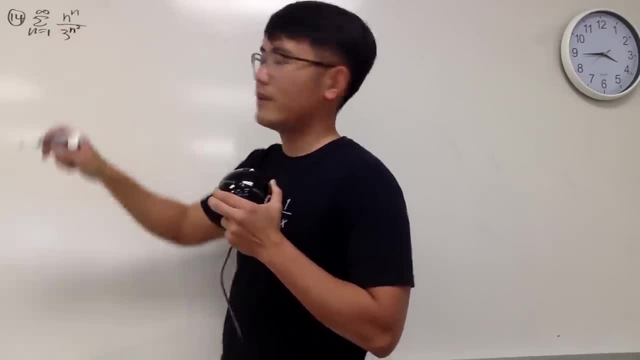 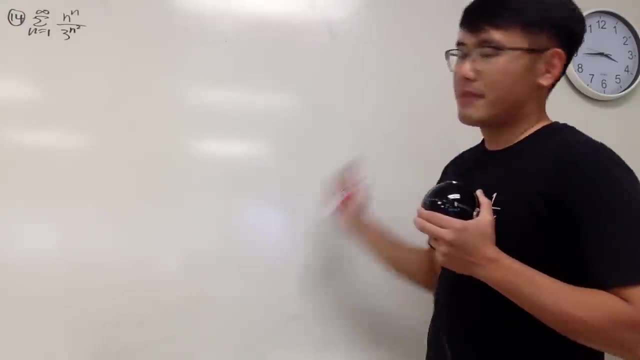 We have 3 to the n, to the second power. First of all, let me tell you, without the little square right here, we can just say that this right here diverges by using the list to show that a n does not approach 0.. 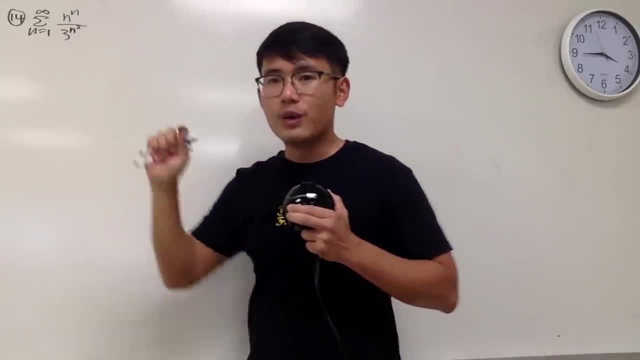 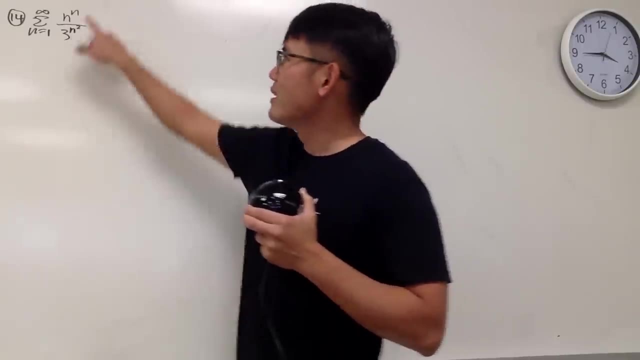 But anyway, we do have the n squared for the power for the 3, so we have more exciting stuff. So let's take a look Both of them. they have the nth power n here and this is n squared. It's a good idea to take the root, the nth root test. 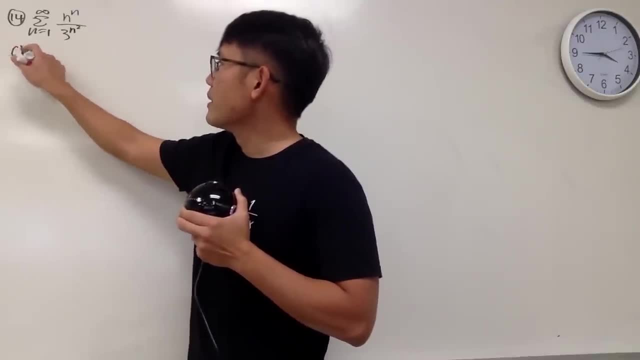 So let's go ahead and check the following right. So, as n goes to infinity, what we are going to do is we'll just take the nth root, and when you do the nth root, you put the absolute value. 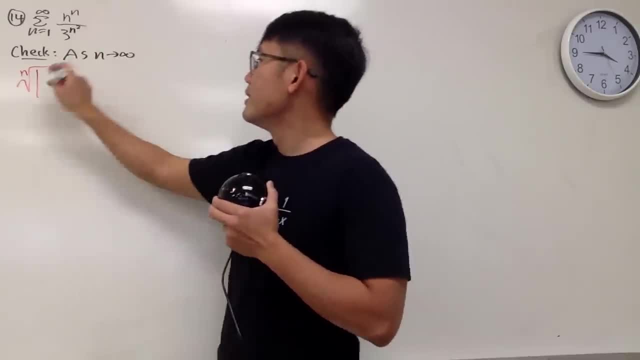 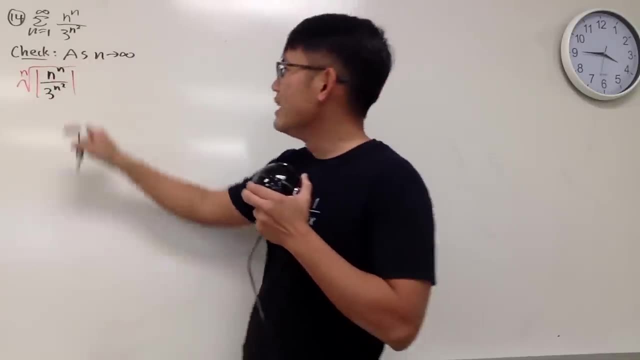 but even though everything is positive, so in this case it doesn't really matter. So we will have n to the n over, 3 to the n squared. We'll check this limit to see what we get right. So let's see. 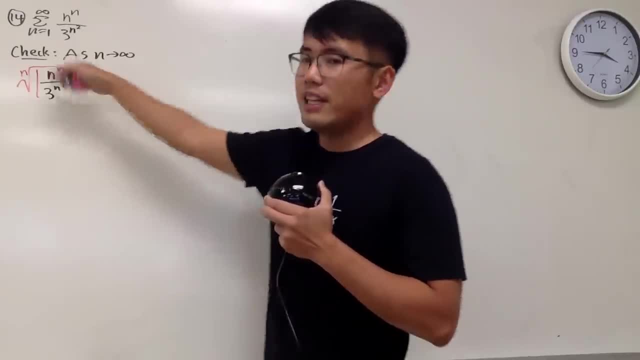 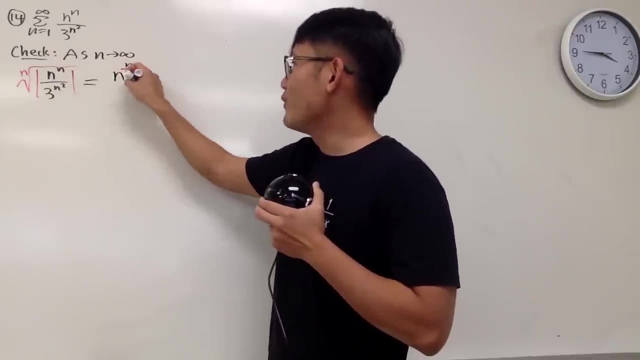 This right here it's just divided by n. Remember, when you take the nth root, just do the top and bottom. So here we have n to the n minus, so over nth power, and then the bottom is 3 to the n squared. 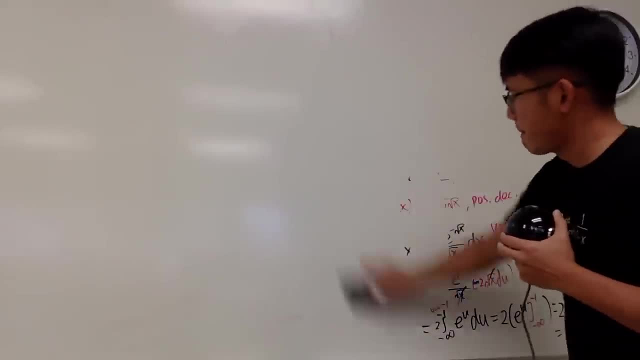 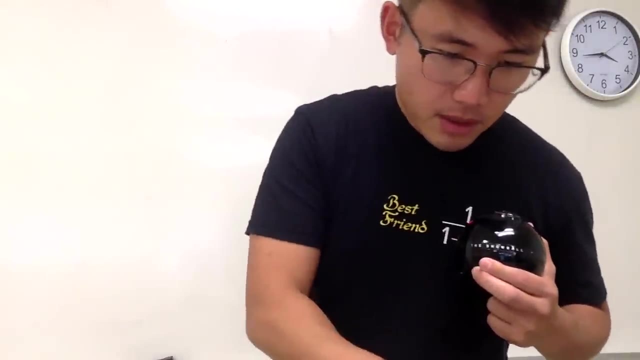 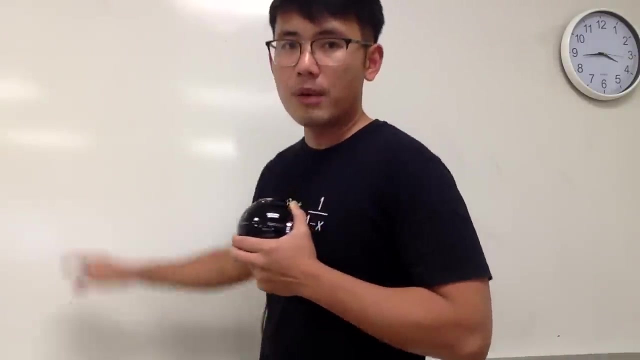 Okay, number 14, top one as well, Let's see. But finally we can do something slightly more computational for the people who like the computational stuff. Number 14.. We are looking at the sum as n goes from 1. 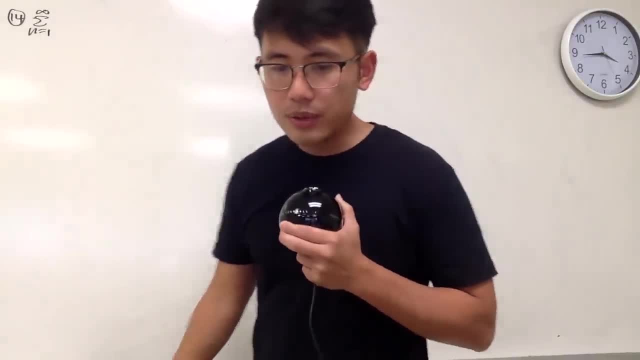 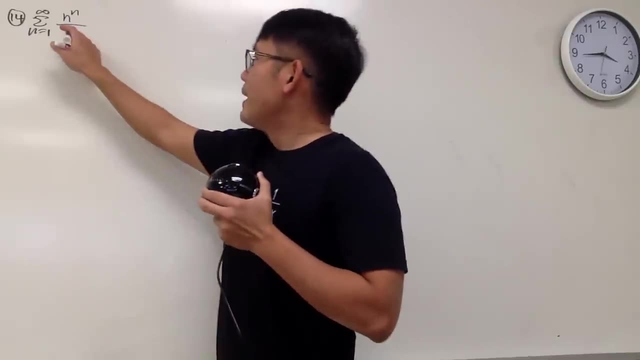 to infinity and we have n to the nth power. Yes, Oh my god, This is n to the nth power. It's like again like the big balls, like Thanos right, But on the bottom we have 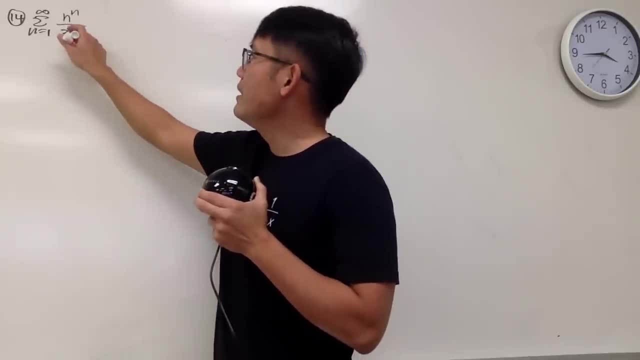 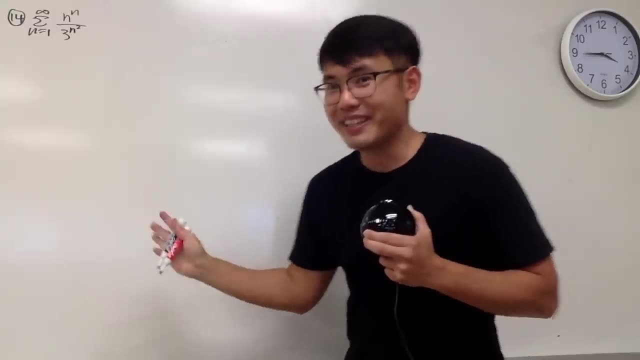 the infinite stone. We have 3 to the n, to the second power. First of all, let me tell you, without the little square right here, we can just say that this right here diverges by using the list to show that an does. 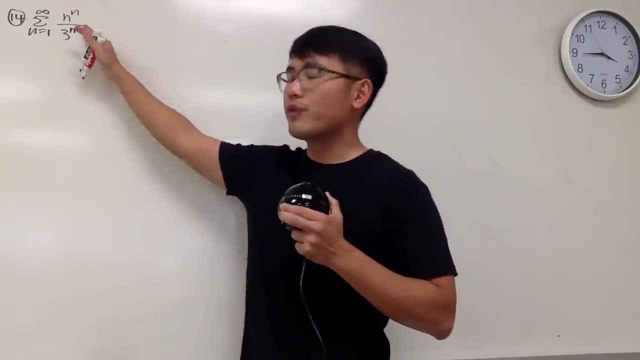 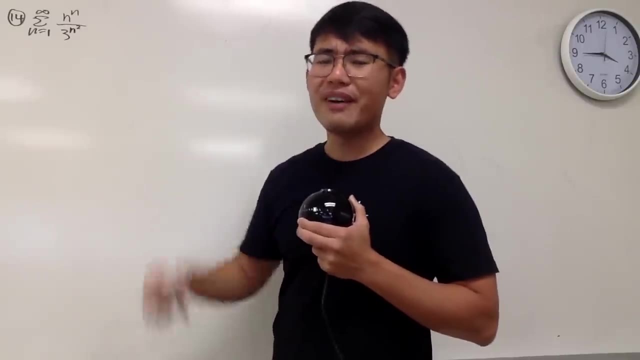 not approach 0.. But anyway, we do have the n squared for the power for the 3, so we have more exciting things going on. So let's take a look. Both of them have the nth power n here, and this is n squared. 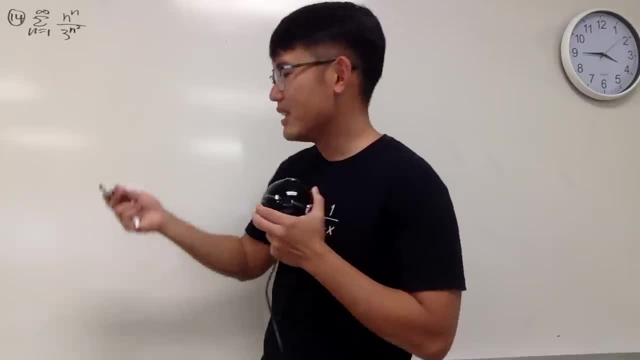 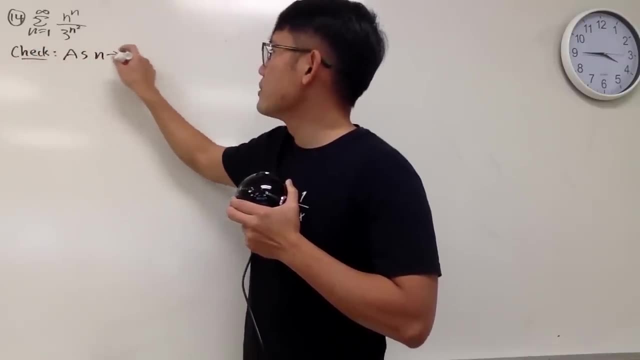 It's a good idea to take the root, the nth root test. So let's go ahead and check the following. Alright, So, as n goes to infinity, what we are going to do is we'll just take the nth root and. 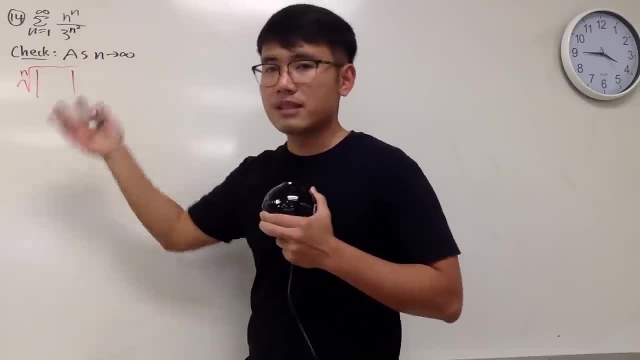 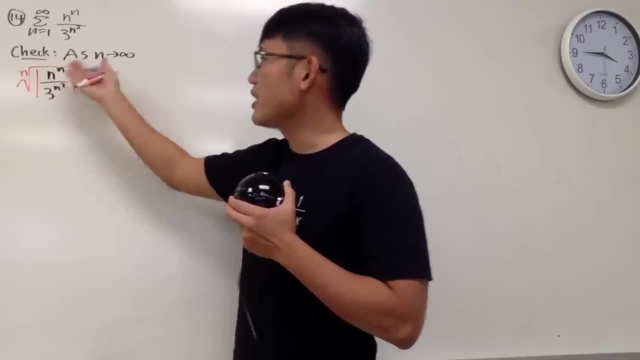 when you do the nth root you put the absolute value, but even though everything is positive, so in this case it doesn't really matter. So we will have n to the n over, 3 to the n squared. We'll check this limit to see what we get. 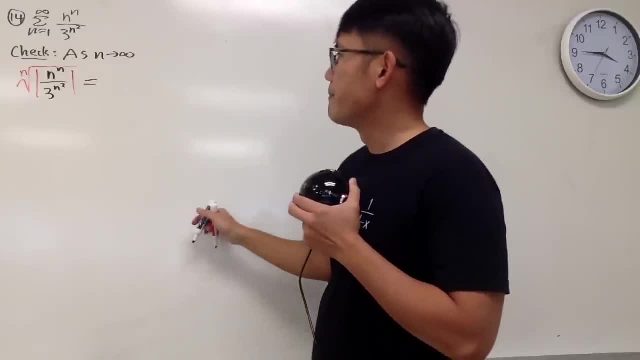 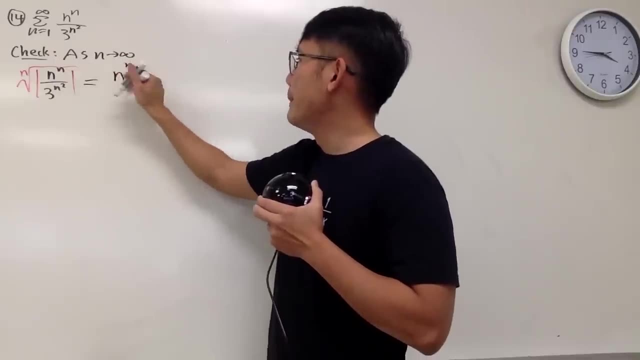 So let's see This right here. it's just divided by n. Remember, when you take the nth root, just do the top and bottom. So here we have n to the n minus over nth power and then the bottom is. 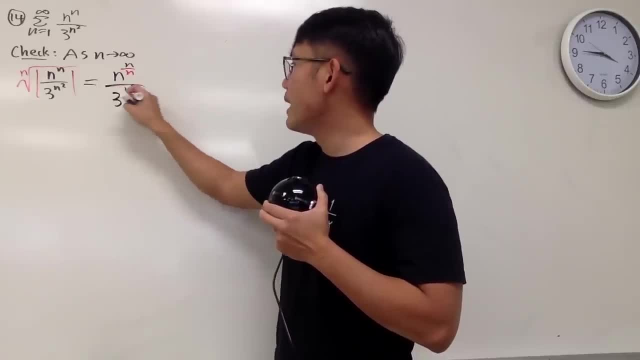 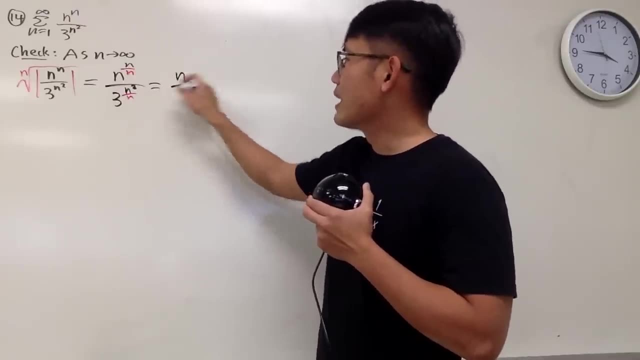 3 to the n, squared but divided by n, right, here And now. here is the beauty of this. Take a look: On the top, it's just n to the first power. On the bottom, we have 3 to the n, like that. 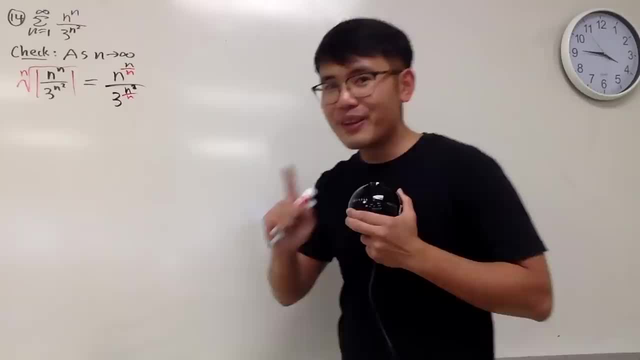 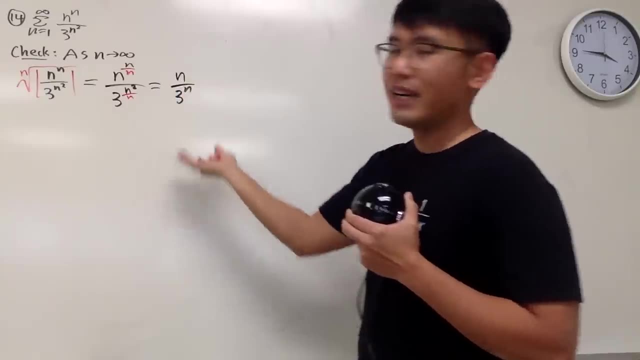 but divided by n. right here, right And now. here is the beauty of this. Take a look: On the top it's just n to the first power. On the bottom, we have 3 to the n, like that. 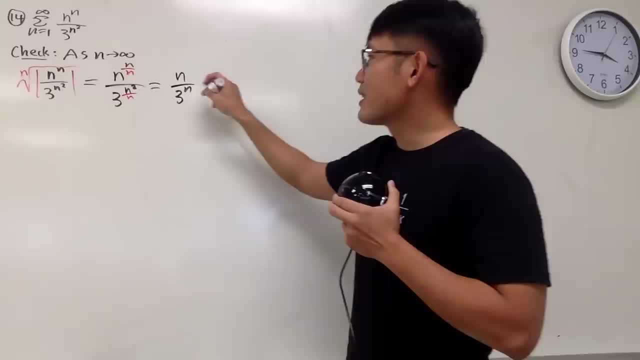 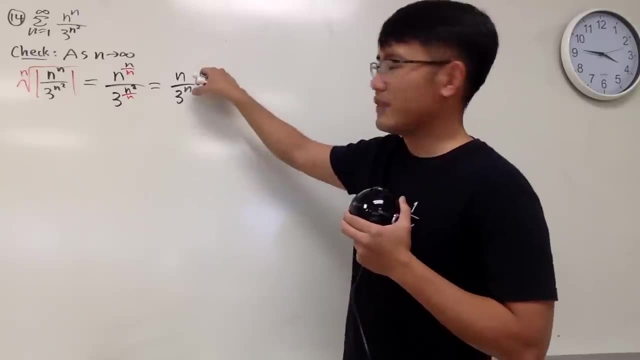 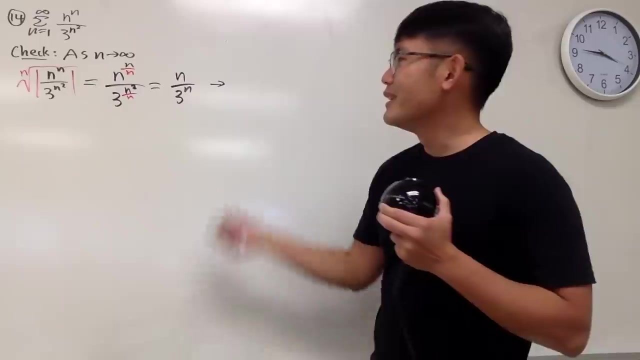 Very nice, huh. And now, as n goes to infinity, can we draw any conclusion? Yes, We have infinity over 3 to the infinity power, but by the least we know, the top infinity is smaller than the bottom infinity. How much smaller. 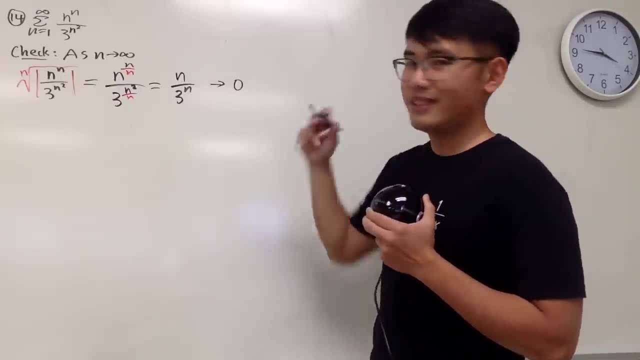 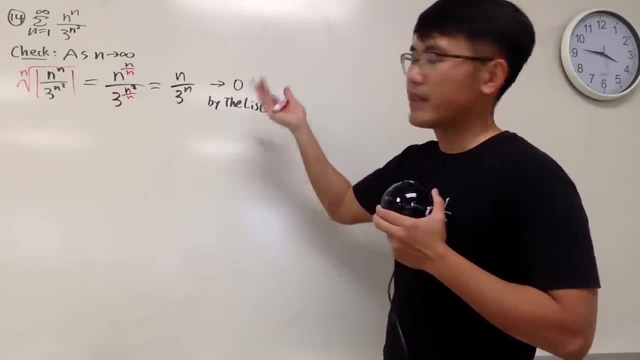 So small. when you divide this by that, you go to 0. And you can put this down and just say: by the least right. So that's pretty much the idea. And remember, here we are using the root test. 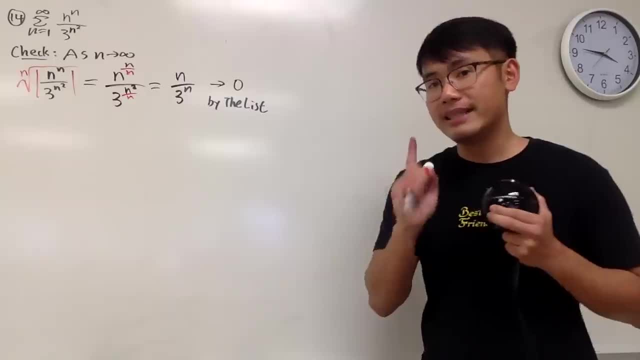 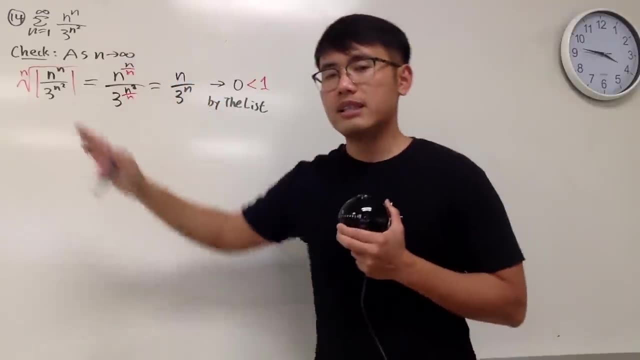 So can the 0 help us? Yes, And you have to compare the 0 with 1.. In this case, if you do the root test, if you end up with 1, unfortunately, we have to do more work for that. 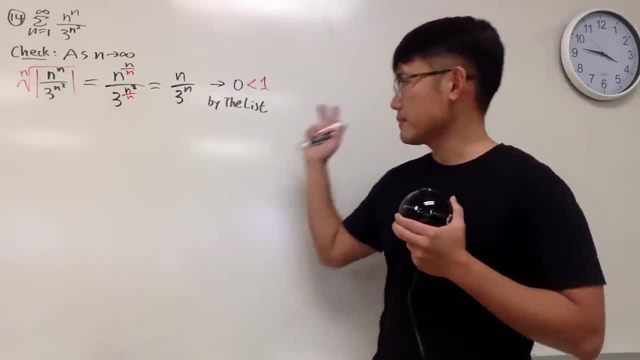 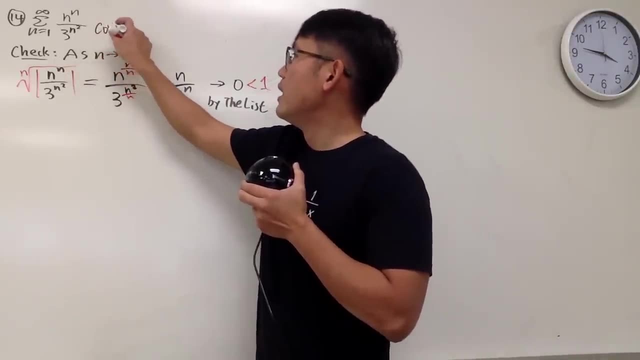 but thankfully this right here is 0,, which is less than 1.. So we can just say by the root test. So this right here actually converges, and we'll just write down by: Unfortunately here we cannot spell. 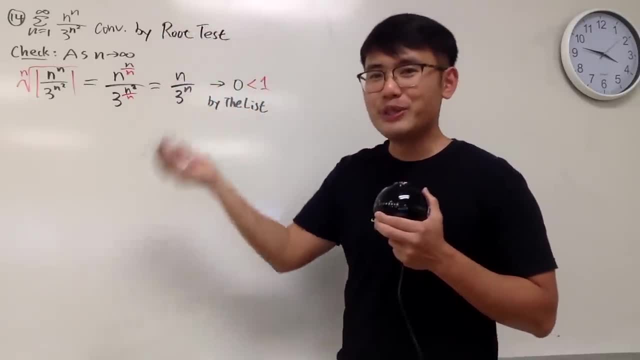 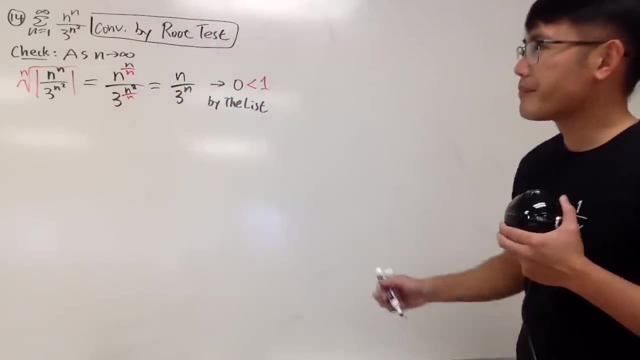 we cannot abbreviate root test because ratio test is also RT, So we'll just spell this out: Converges by the root test, just like that, right. So that's it, which is pretty good, pretty good, pretty good. 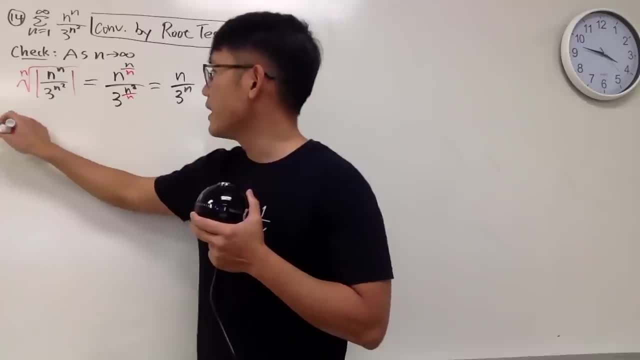 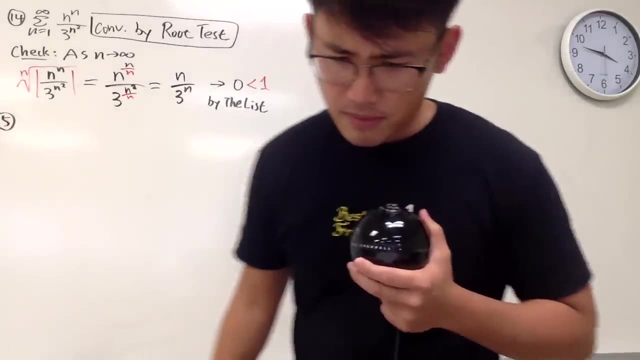 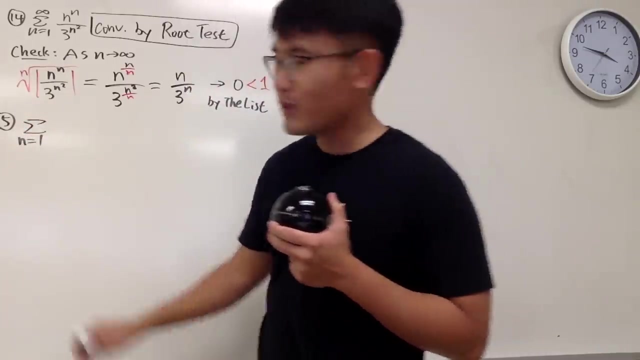 And of course, we'll continue, continue, continue. Number 15.. Number 15.. Okay, My God, another big one. Now we have the sum, as n goes from 1 to infinity, and we have n to the nth power. 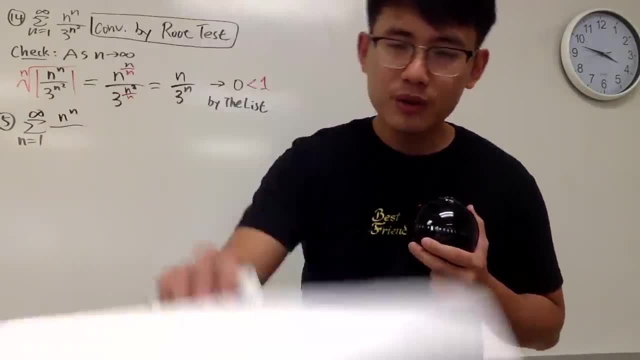 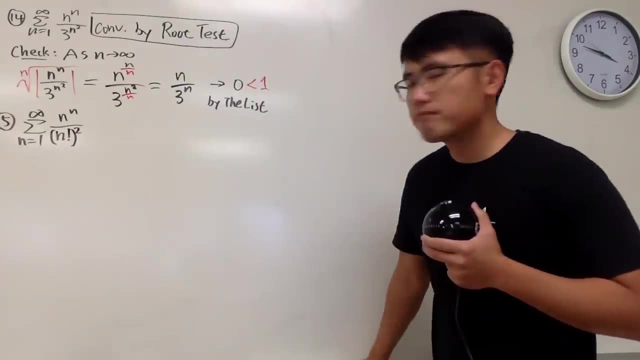 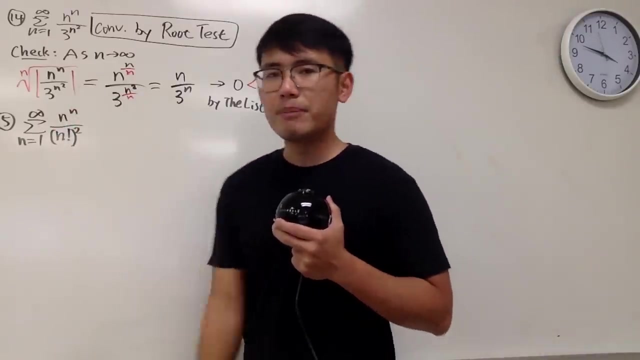 over n factorial square. Oh my God n factorial square. Hmm, are you guys ready for this? Okay, If we take the nth root, okay, that can take care of that power nicely. but the problem is that when we have factorials, 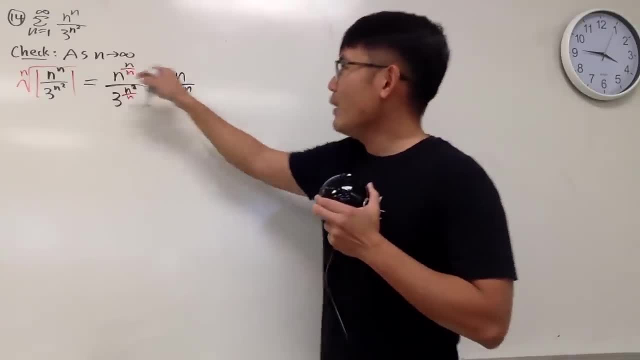 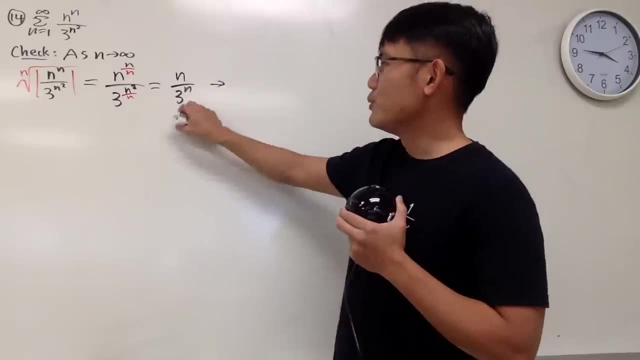 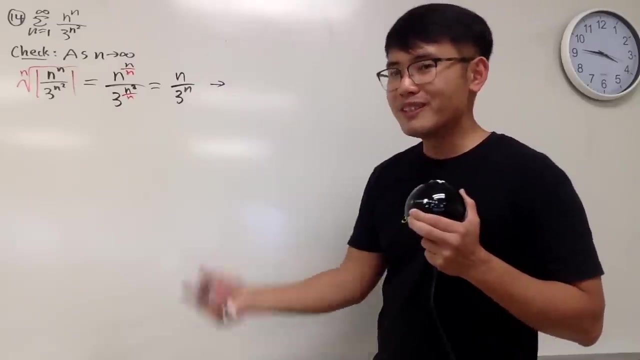 Very nice, huh. And now, as n goes to infinity, can we draw any conclusion? Yes, We have infinity over 3 to the infinity power, but by the list we know the top infinity is smaller than the bottom infinity. How much smaller. 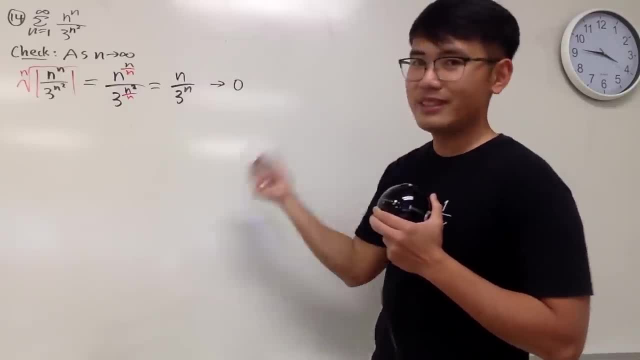 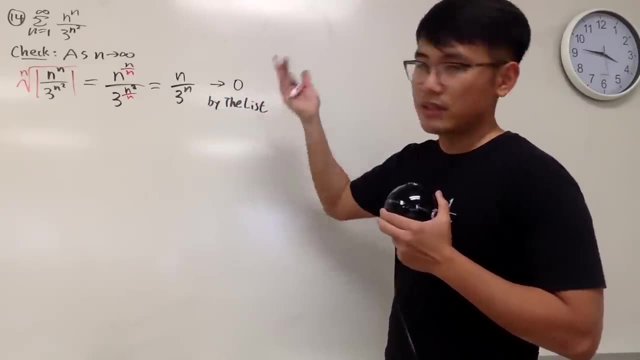 So small. when you divide this by that, you go to 0. And you can put this down and just say: by the list, Right? So that's pretty much the idea. And remember, here we are using the root test. so 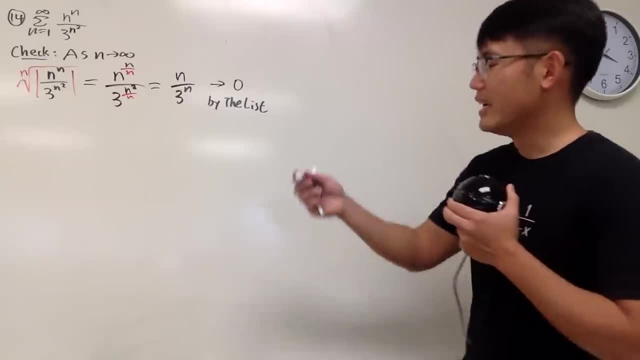 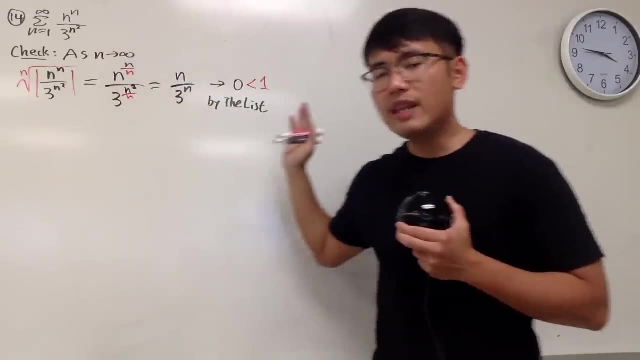 can the 0 help us? Yes, And you have to compare the 0 with 1.. In this case, if you do the root test, if you end up with 1, unfortunately, we have to do more work for that, but 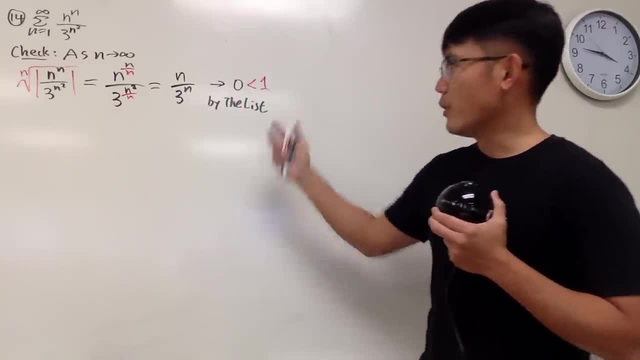 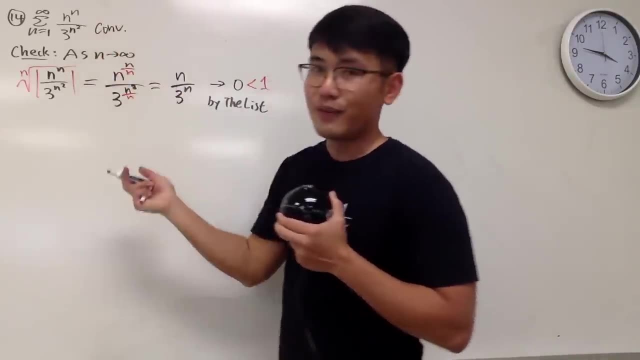 thankfully this right here is 0,, which is less than 1, so we can just say by the root test. So this right here actually converges, and we'll just write down by: unfortunately here we cannot spell, we cannot. 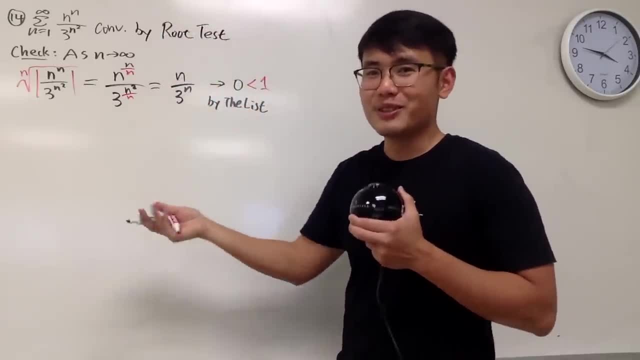 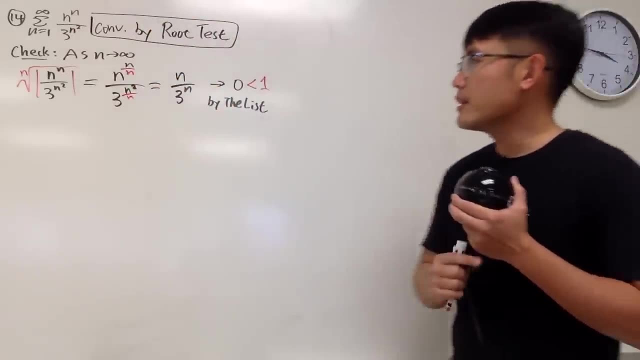 abbreviate root test, because ratio test is also RT, So we'll just spell this out: Converges by the root test, Just like that, Right? So that's it, Which is pretty good, pretty good, pretty good. 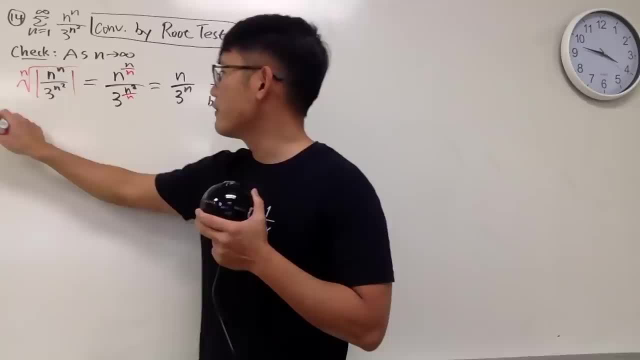 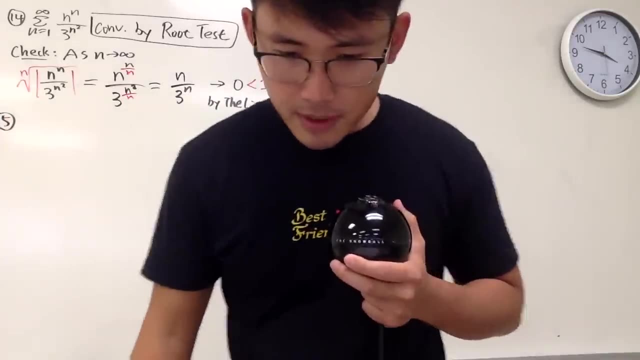 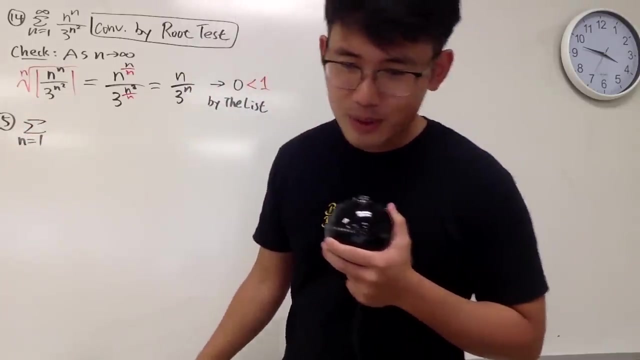 And of course, we'll continue, continue, continue. Number 15.. Number 15.. Okay, My god, Another big one. Now we have the sum as n goes from 1 to infinity, and we have n to the nth power over. 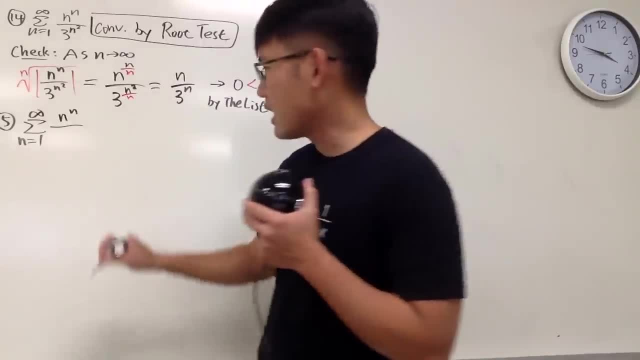 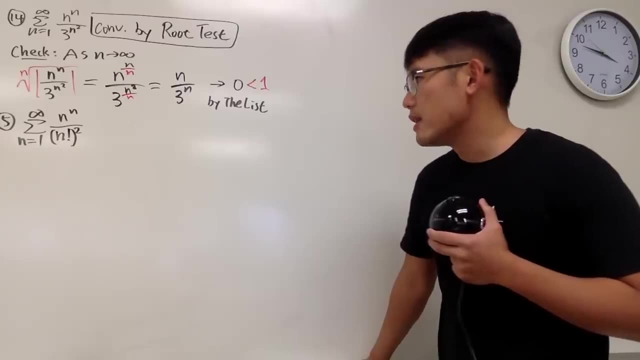 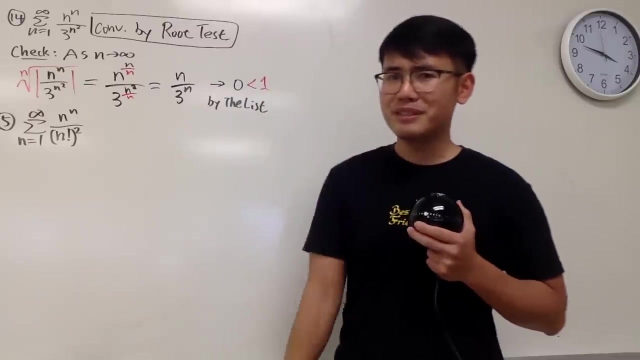 n factorial squared. Oh my god n factorial squared. Hmm, Are you guys ready for this? Okay, If we take the nth root, okay, they can take care of that power nicely. but the problem is that when we have factorials, 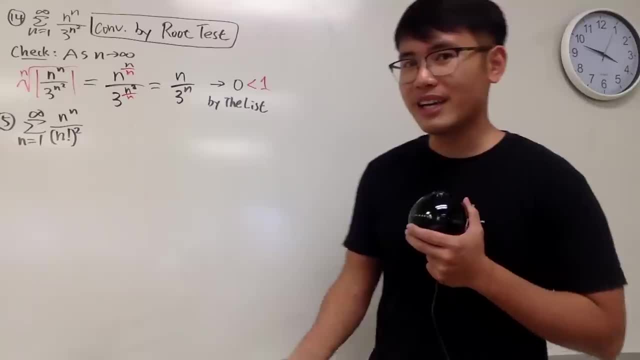 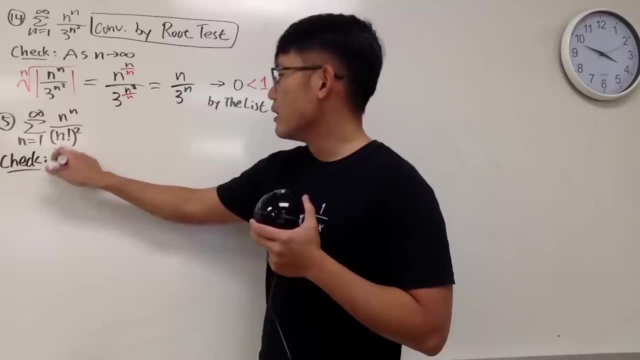 not so much, huh. So here it's a good idea to use the ratio test. So we'll just use the ratio test, and this is the check that we will have to do Again. take the limit, as n goes to infinity. 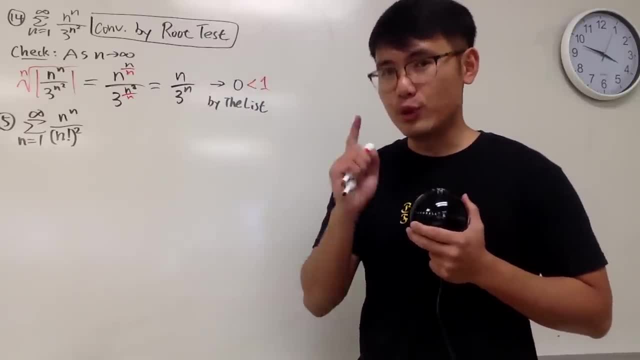 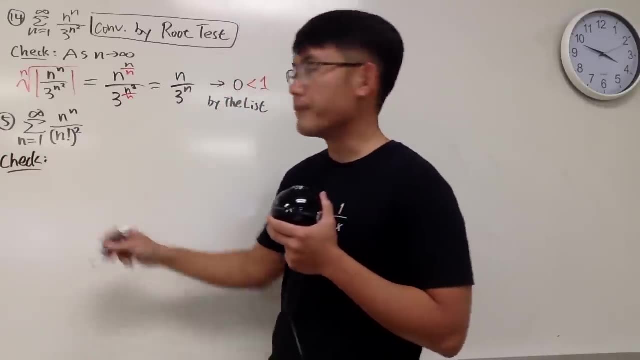 not so much, huh. So here it's a good idea to use the ratio test. So we'll just use the ratio test, and this is the check that we will have to do Again. take the limit, as n goes to infinity. 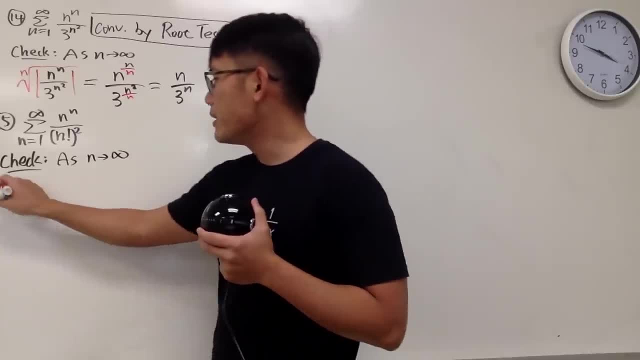 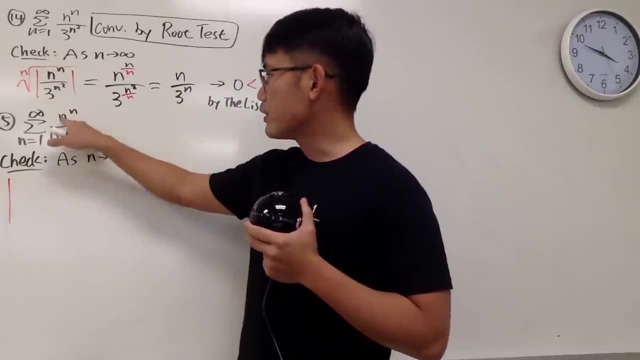 and for the ratio test, just do the following: First of all, open absolute value and you are going to put down a n plus 1, right, which is just put down n plus 1 to all the n's right here. 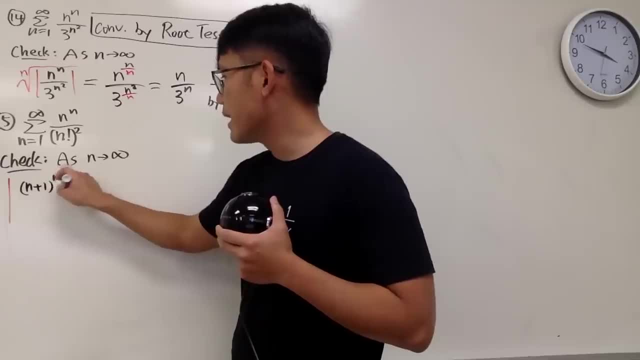 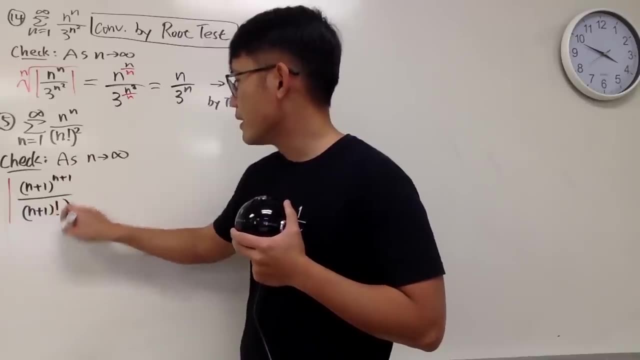 So in another word, we get n plus 1 raised to the n plus 1 power over n plus 1 factorial, like this, and then you do the square on the outside, So n plus 1 and factorial, and then just like that. okay. 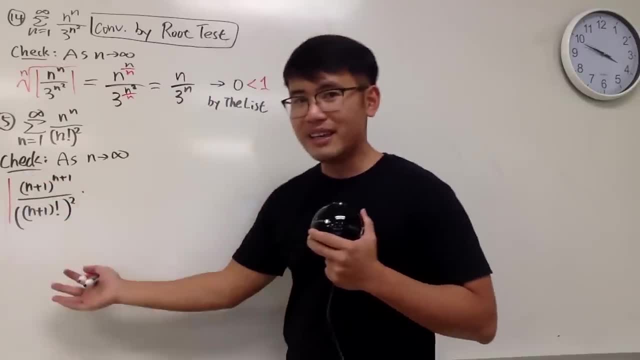 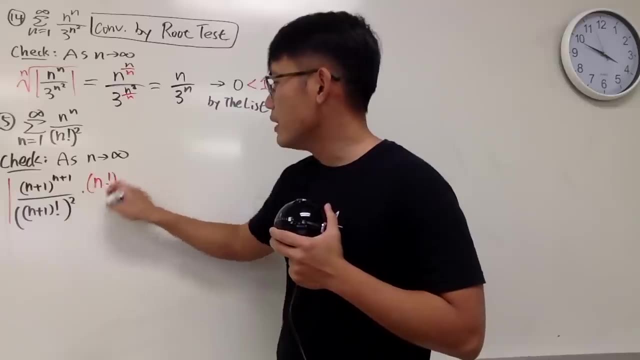 And then this is a n plus 1. You have to divide it by a n, and divide it by a n is the same as looking at this and you do the reciprocal. so we get n factorial and then we square that. 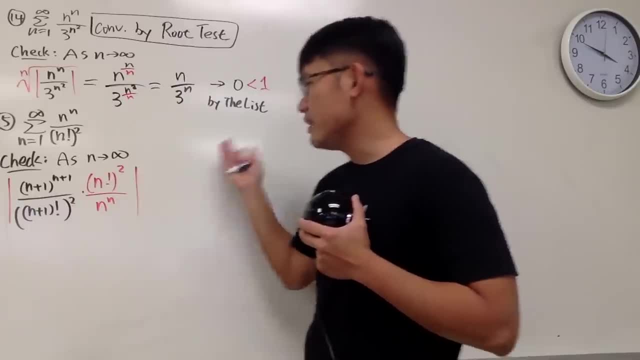 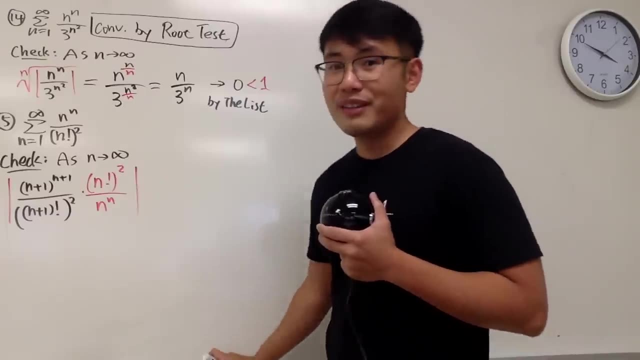 and then we divide it by n to the n's power, like that in the absolute value. So this right here is very nice. Now we are going to break down the factorials and also the powers to see what's up with that right. 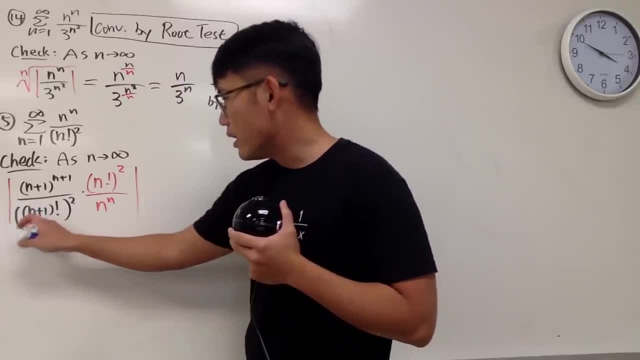 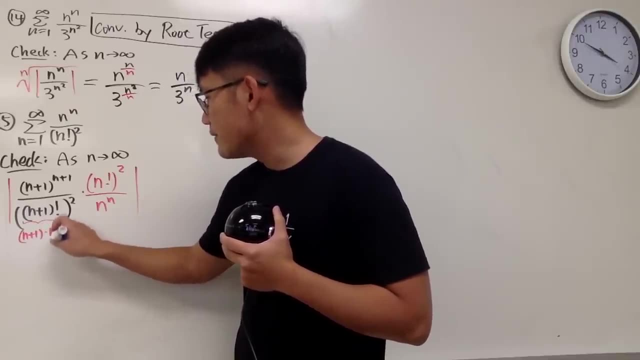 Okay, First of all, this right here: n plus 1 factorial is the same as saying n plus 1 times n factorial. like this right, You start with the parentheses inside and then you go down by 1, like that. 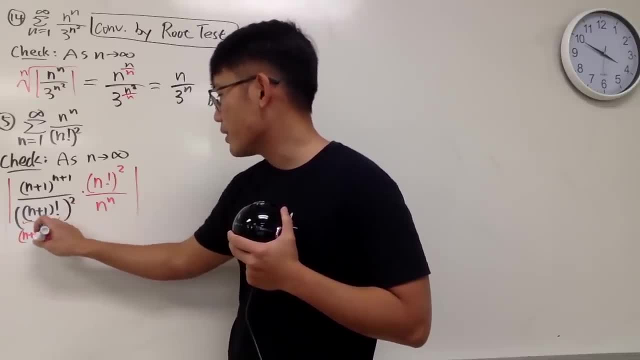 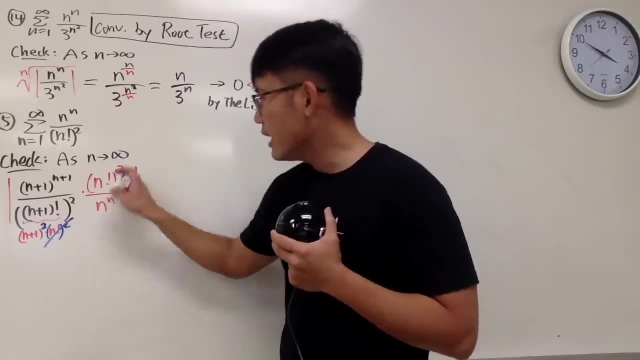 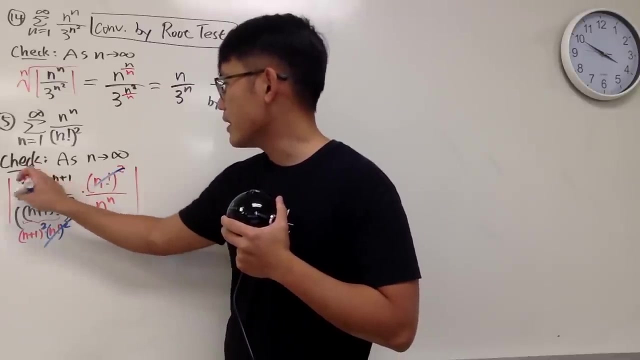 and you have this, the square, so you have to put down the square here and here right And notice the n factorial square, this and that can be cancelled. so that's very nice. Now continue Right here. this, right here. this is the same as saying: 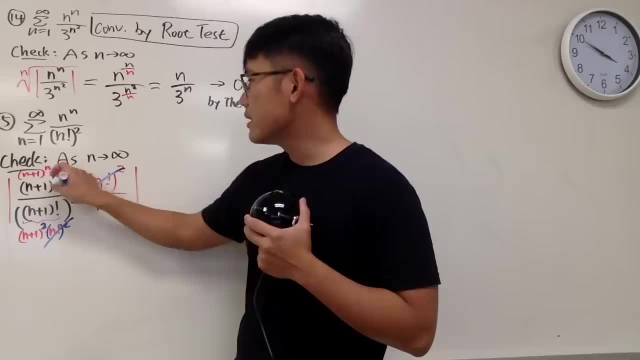 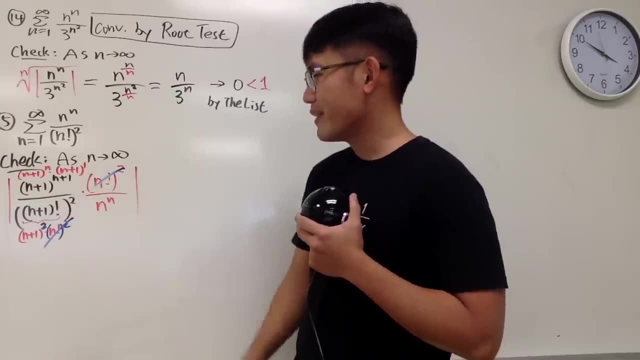 n plus 1 to the n's power times, n plus 1 to the first power, so that you can, if you multiply them, you can combine the powers together, And the beauty is that n plus 1 to the first power can be cancelled with one of these. 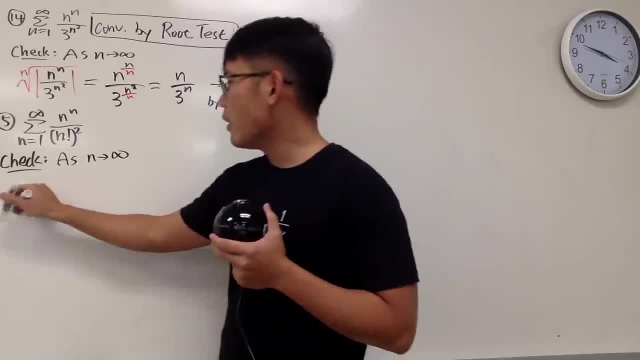 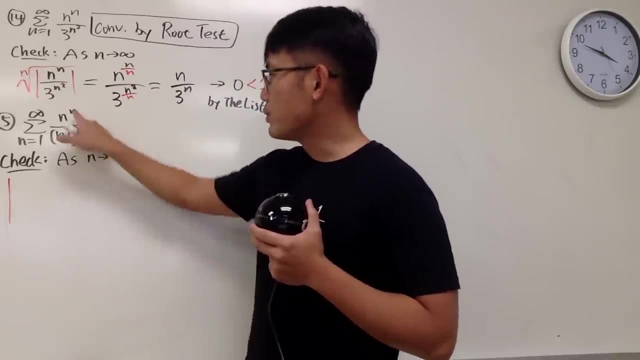 and for the ratio test, just do the following: First of all, open absolute value and you are going to put down a n plus 1, right, which is just put down n plus 1 to all the n's right here. 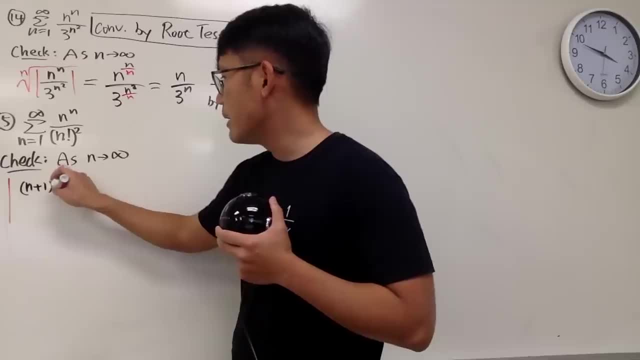 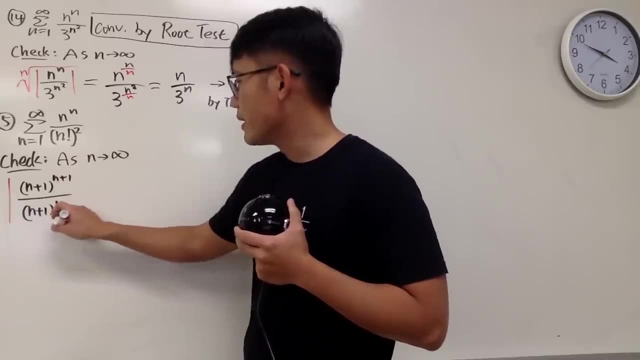 So in another word, we get n plus 1 raised to the n plus 1 power over n plus 1 factorial, like this, and then you do the square on the outside, So n plus 1 factorial and then just like that. okay. 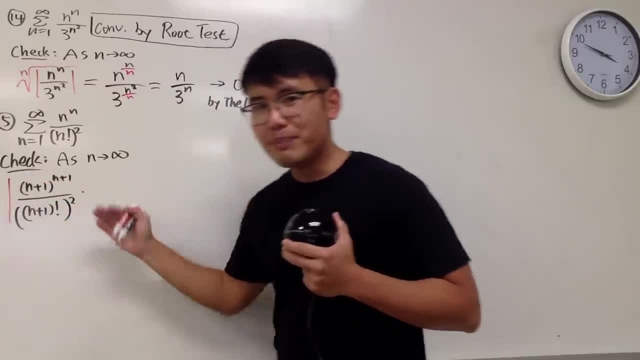 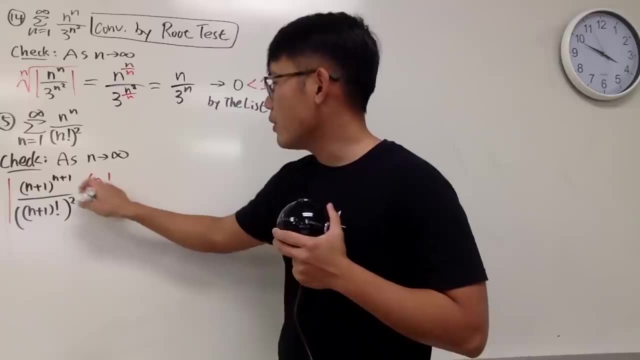 And then this is a n plus 1. You have to divide it by a n, and divide it by a n is the same as looking at this, and you do the reciprocal. so we get n factorial and then we square that and then we divide it by. 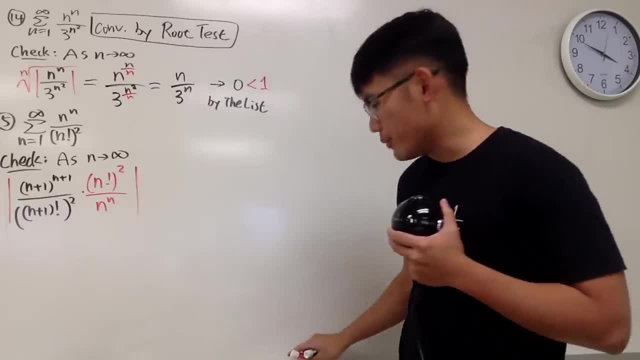 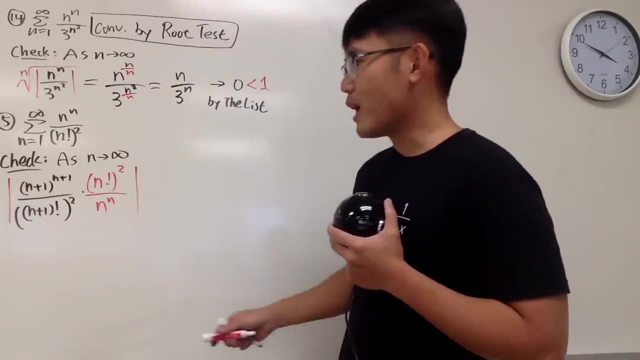 n to the n's power, like that in the absolute value. So this right here is very nice. Now we are going to break down the factorials and also the powers to see what's up with that, right Okay. 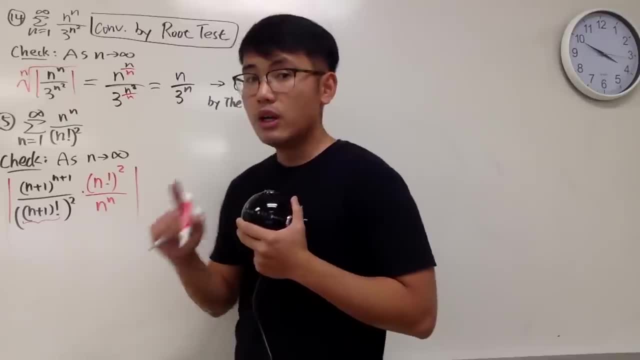 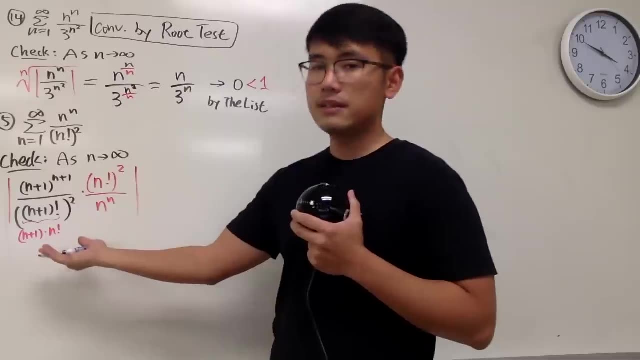 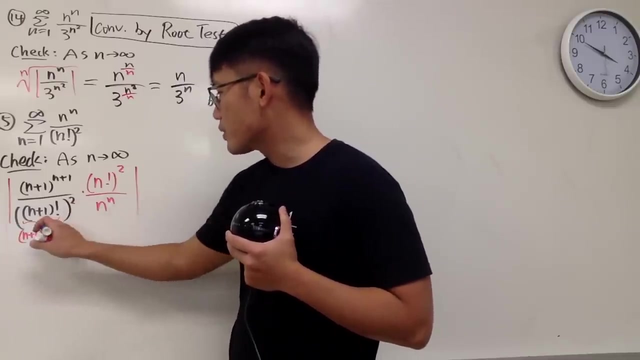 First of all, this right here: n plus 1 factorial is the same as saying n plus 1 times n factorial. like this right, You start with the parentheses inside and then you go down by 1, like that, and you have this the square. so you have to. 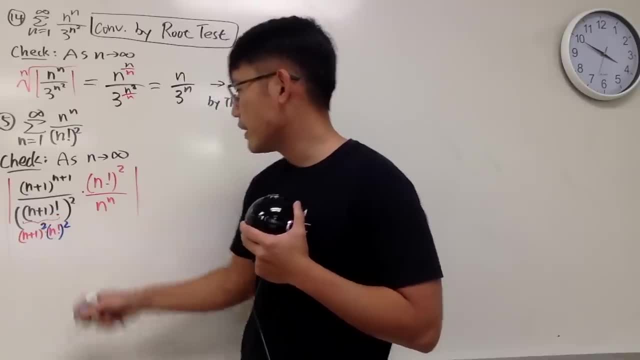 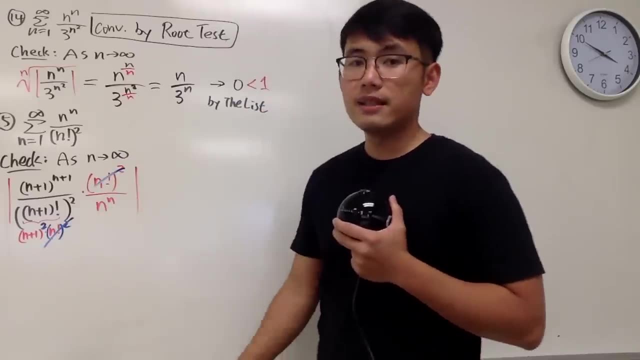 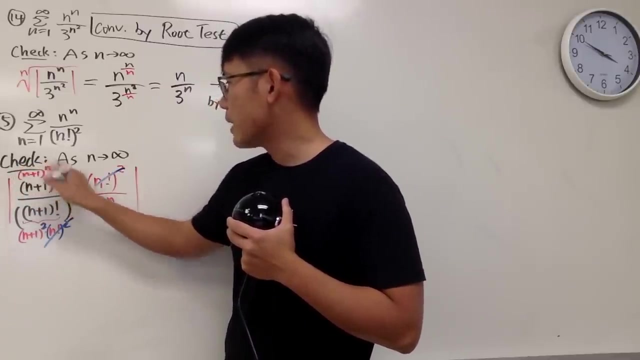 put down the square here and here Right, And notice the n factorial square, this and that can be cancelled. so that's very nice. Now continue Right here. this, right here. this is the same as saying n plus 1 to the n's power. 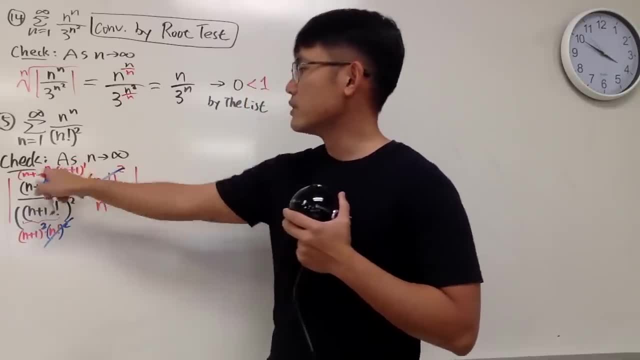 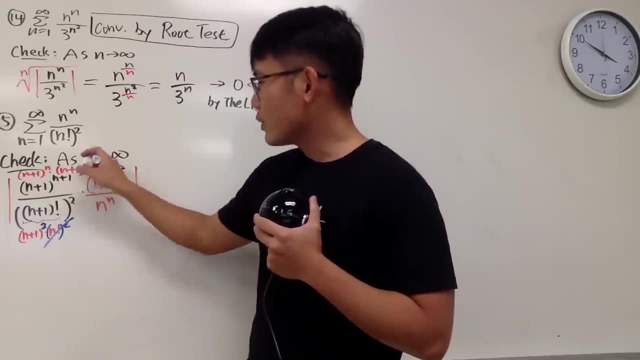 times n plus 1 to the first power, so that you can, if you multiply them, you can combine the powers together, And the beauty is that n plus 1 to the first power can be cancelled with one of these, so this becomes the first power, right there. 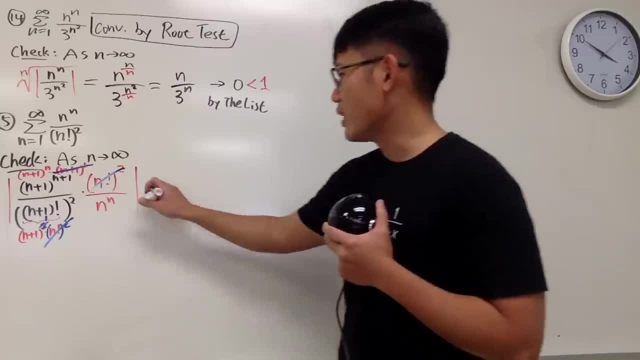 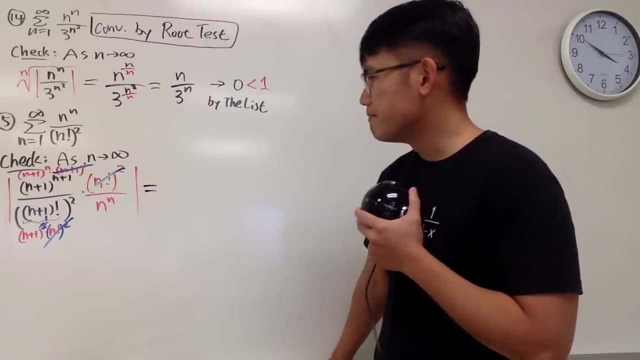 So that's pretty much the most we can do. huh, And now everything's positive, so we don't need the absolute value anymore, and let's see what else can we do. Hmm, Okay, This guy and that guy. 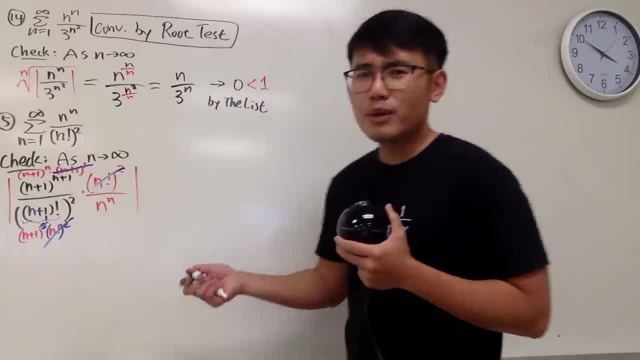 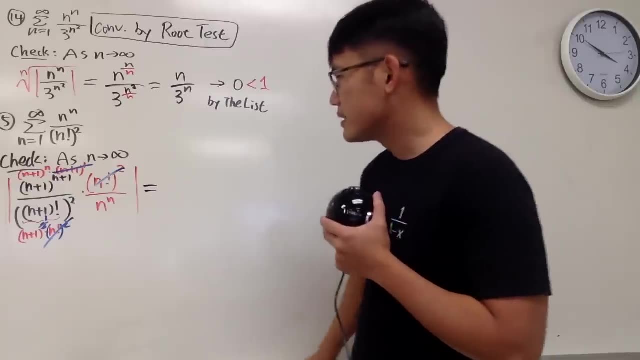 so this becomes the first power right there. So that's pretty much the most we can do, huh, And now everything's positive, so we don't need the absolute value anymore and let's see what else can we do. Hmm. 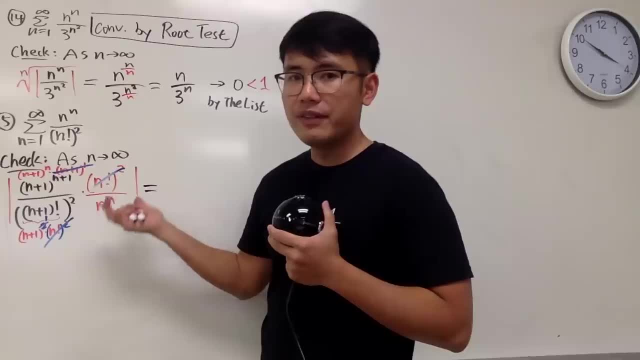 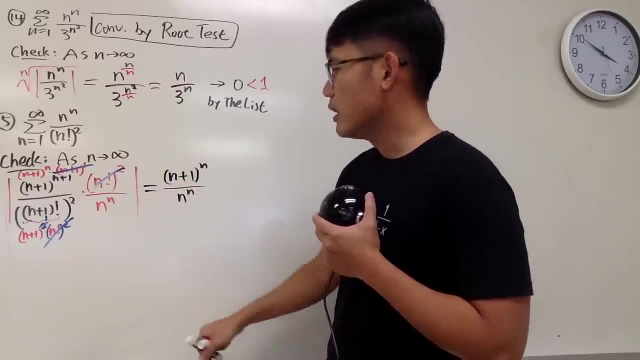 Okay, This guy and that guy, they all have the n's power. so I will put them down together: first n plus 1 to the n's power, over n to the n's power, and then right here we have n plus 1,. 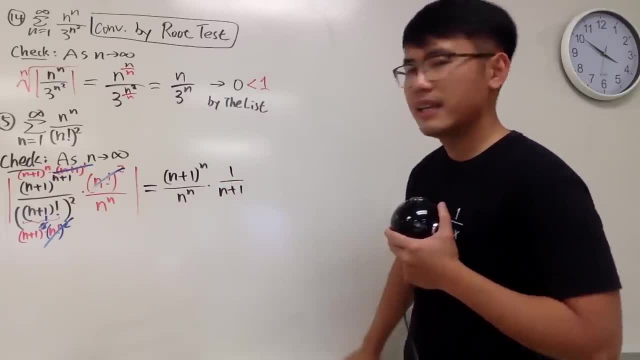 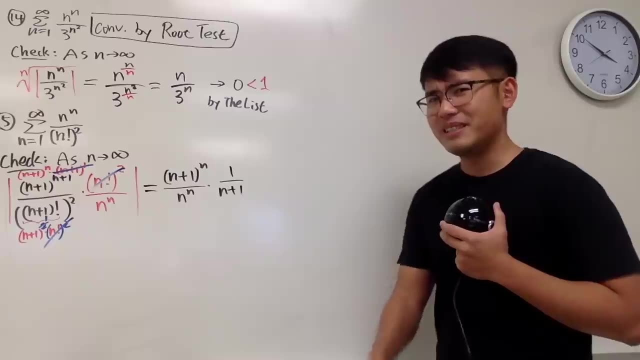 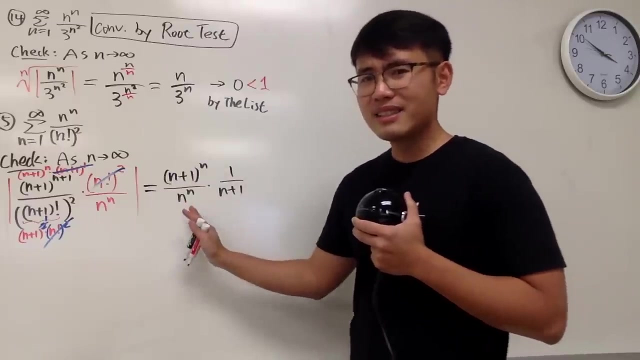 so we'll multiply by 1 over n plus 1, like that. Okay, So far, so good. Let's see, Technically, what's the limit, as n goes to infinity of this, This is not 1, okay for the limit. 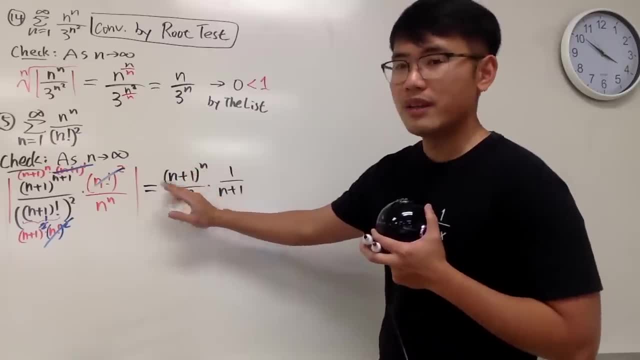 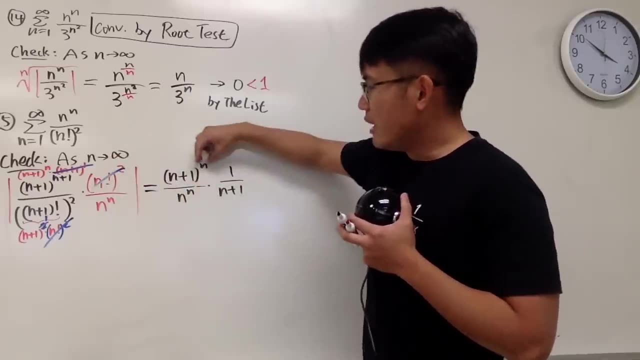 Even though you might attempt to just cover the 1 right here and say this is n to the n's power over n to the n's power, but it's actually not true, because n is approaching infinity and you have the power right here. 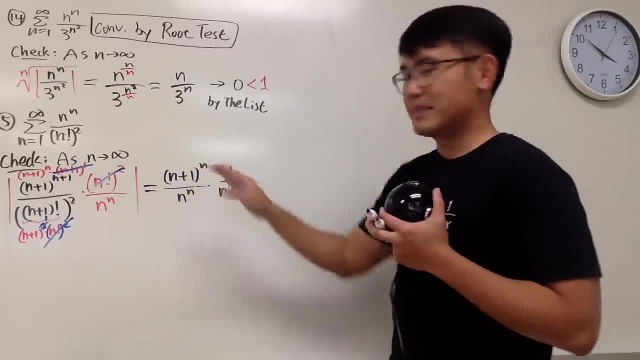 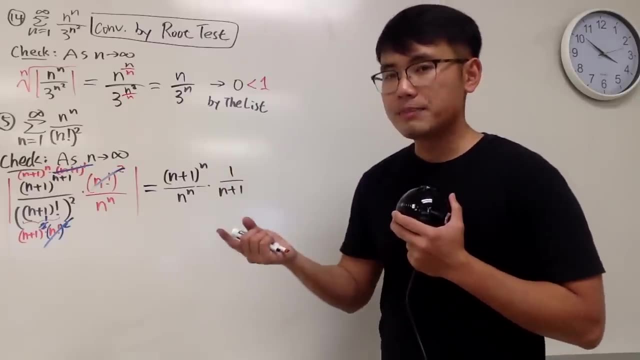 So technically you have infinitely many terms on the top, so that's, if you ever expand that, so you cannot do that Now. this is where the fact kicks in. Both of them are of to the n's power, so let's do some more algebra. 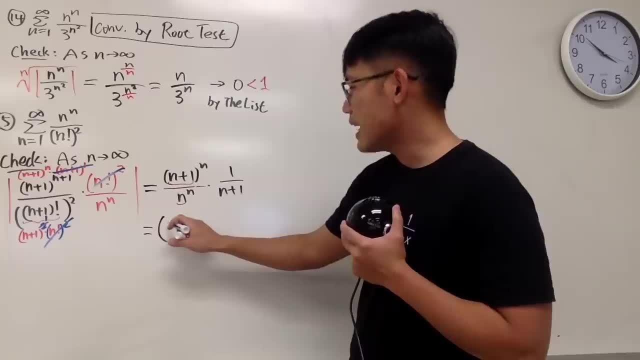 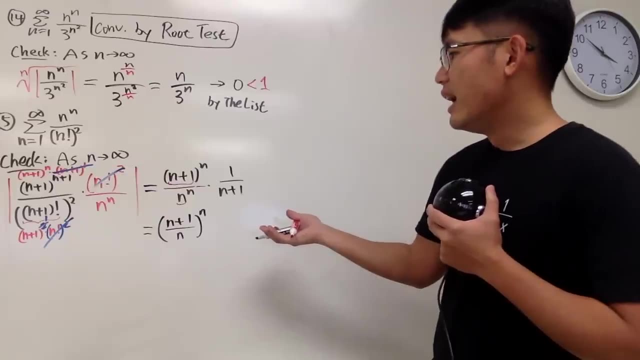 We can write this down as this over that inside, so n plus 1 over n, and then raise to the n's power like that. And I notice maybe you want to subtract the power, but don't do it And then just leave this on the outside. 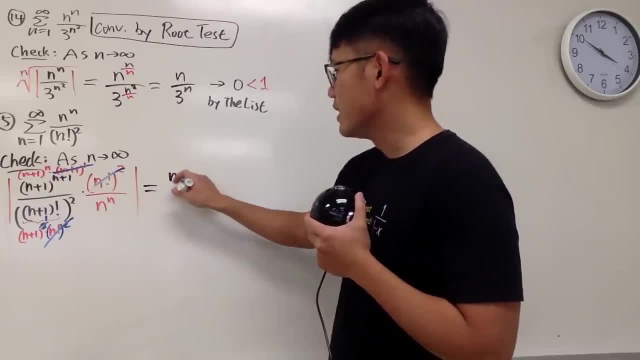 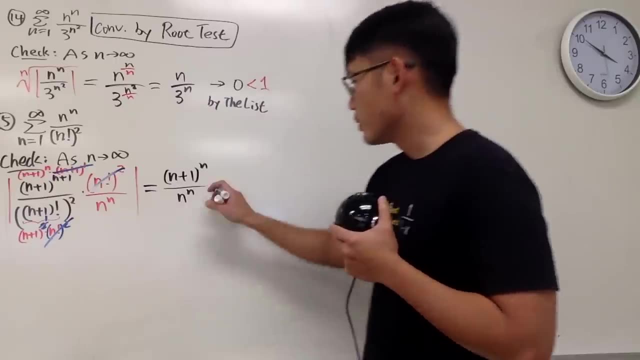 they all have the n's power, so I will put them down together: first n plus 1 to the n's power, over n to the n's power, and then right here we have n plus 1, so we'll multiply by 1 over. 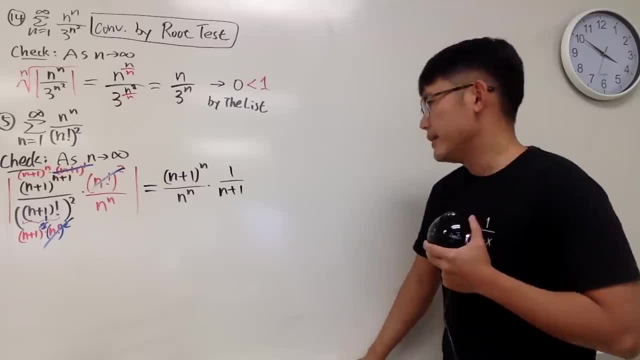 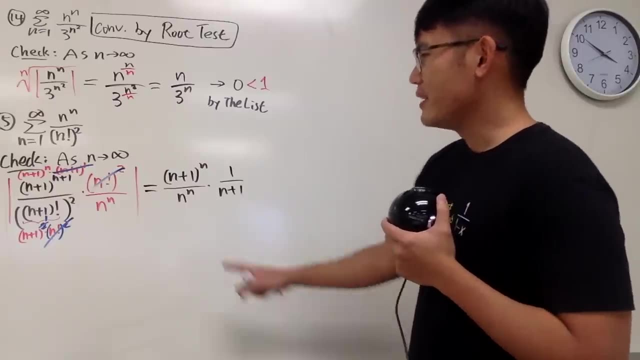 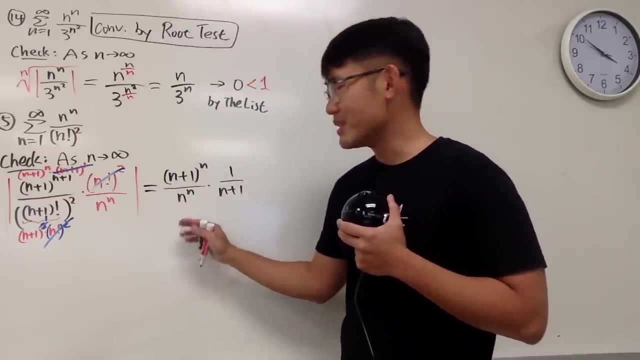 n plus 1, like that. Okay, So far, so good. Let's see, Technically, what's the limit, as n goes to infinity of this, This is not 1, okay for the limit, Even though you might attempt to. 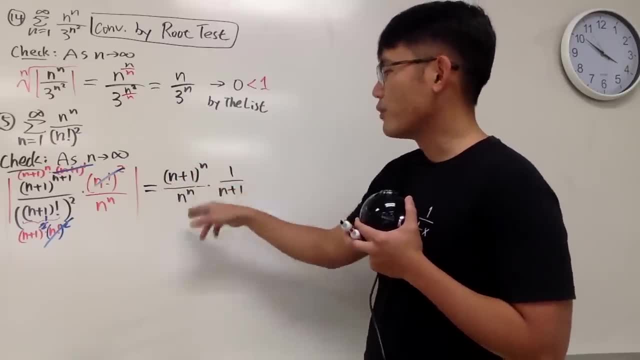 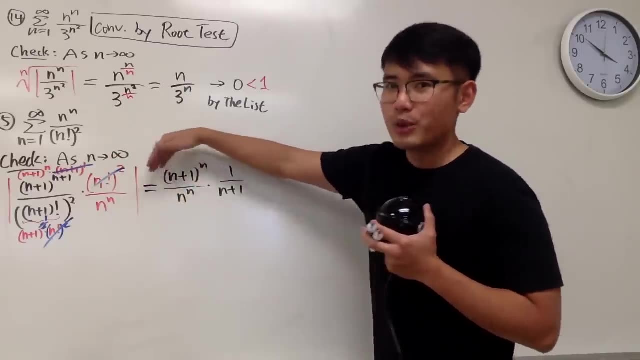 just cover the 1 right here and say this is n to the n's power over n to the n's power. but it's actually not true, Because n is approaching infinity and you have the power right here, So technically you have infinitely many terms on the top. 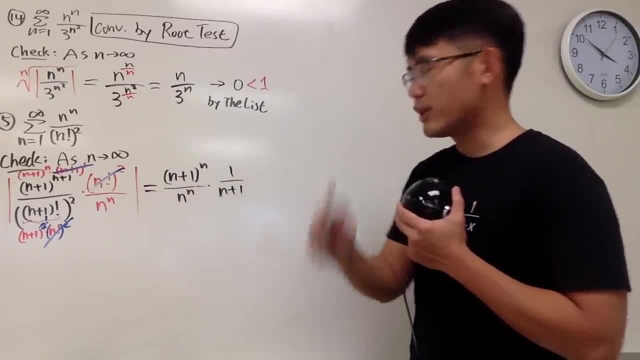 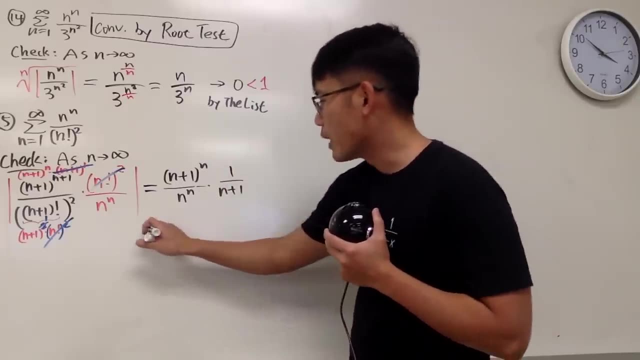 So that's if you ever expand that. So you cannot do that Now. this is where the fact kicks in. Both of them are off to the n's power, so let's do some more algebra. We can write this down as this: over that. 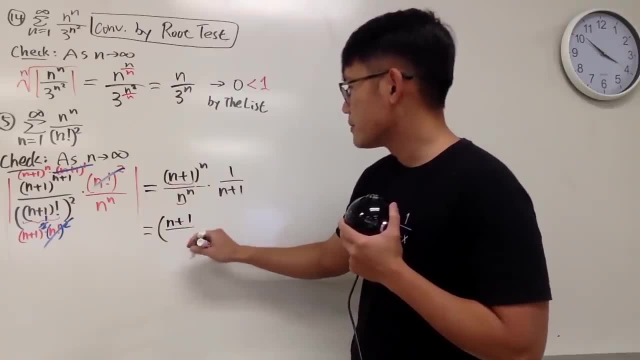 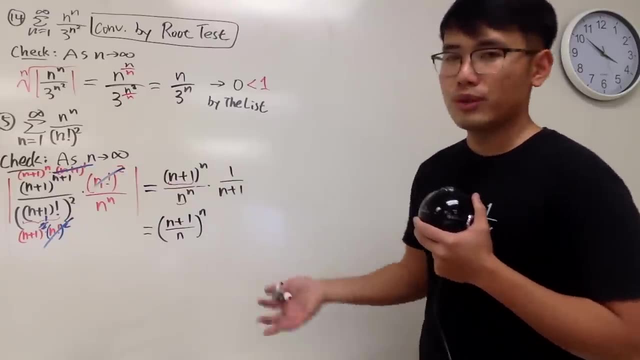 inside, so n plus 1 over n and then raise to the n's power, like that. And I notice, maybe you want to subtract the power, but don't do it. Just leave this on the outside. you will see why I'm doing this. alright, 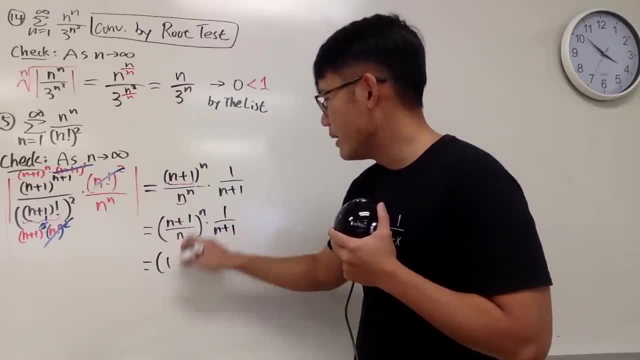 Now, of course, you can just simplify this: n over n is just 1, and you have 1 over n to the n's power, like that. And take a look what this is. Take a look what this is. Very cool, huh. 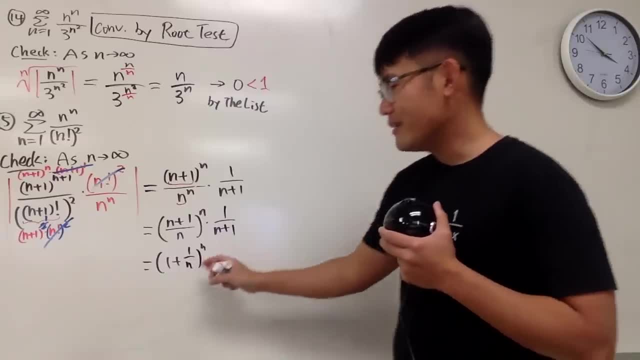 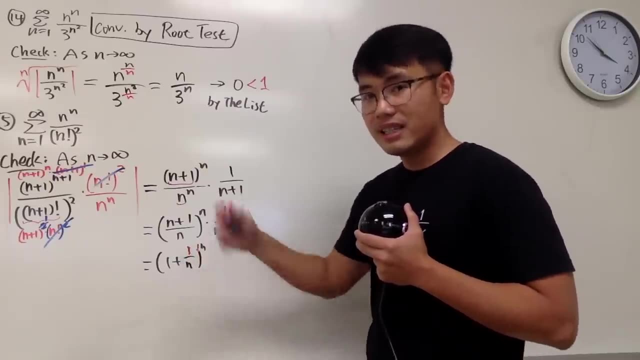 This is what. This is the special number e, right, And of course, if you want to quote the fact, a is 1 and it's positive 1 and b is also positive 1.. So this guy gives you e to the. 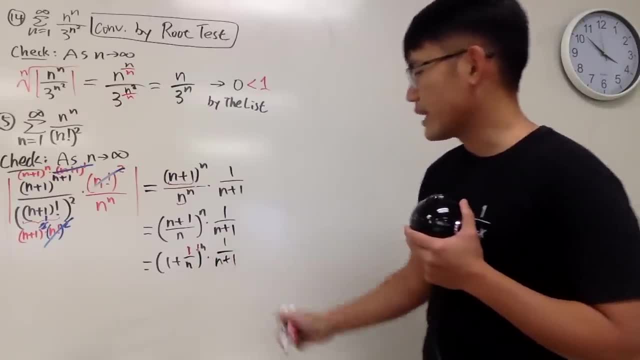 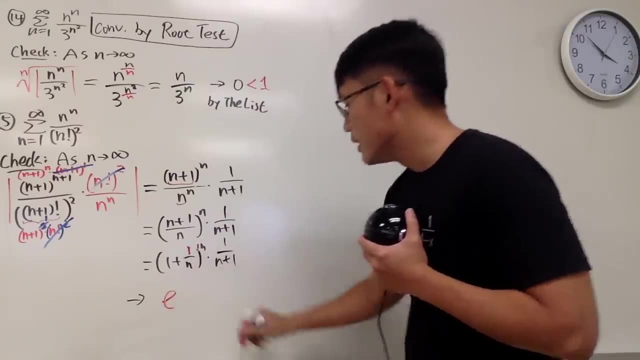 first power n times 1 over n plus 1, like that. Now take the limit Again. this right here is the definition of e, where you can quote the fact: It's just e, but this right here is 1 over infinity. 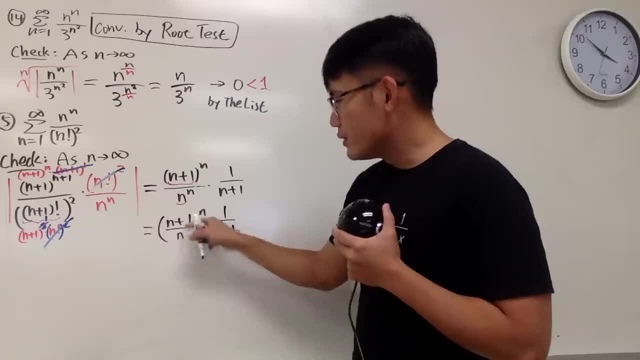 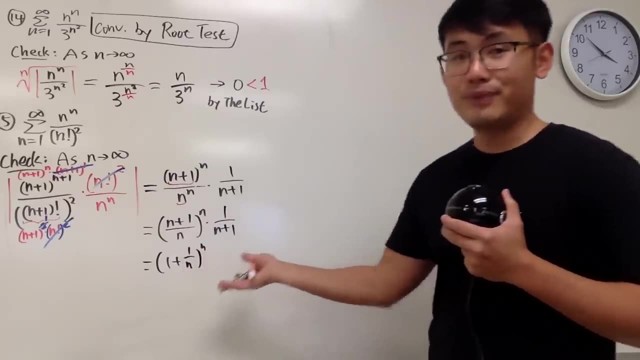 you will see why I'm doing this. alright, Now of course, you can just simplify this: n over n is just 1, and you have 1 over n to the n's power, like that. And take a look what this is. 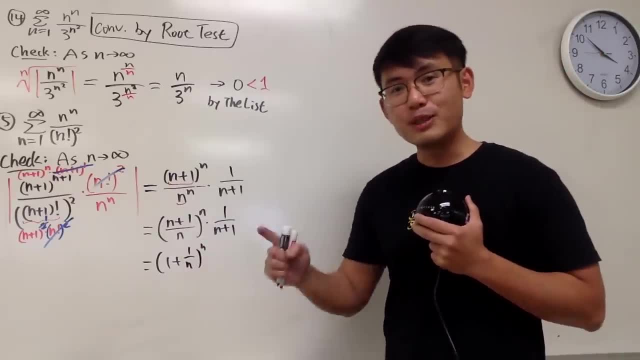 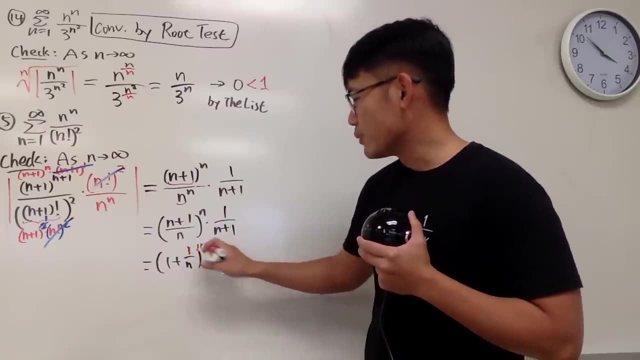 Take a look what this is. Very cool, huh? This is what This is. the special number e, right. And of course, if you want to quote the fact, a is 1, and it's positive 1, and b is also positive 1.. 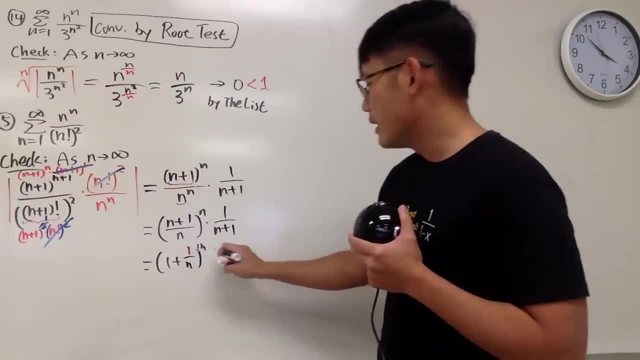 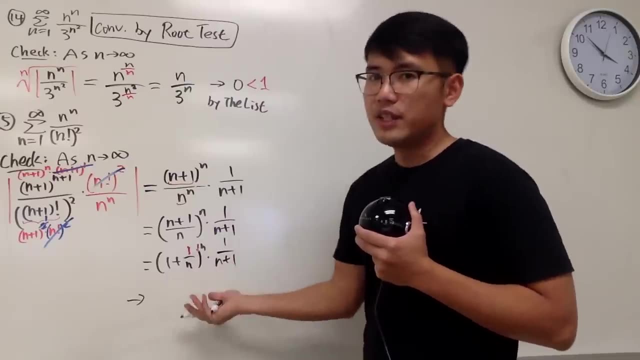 So this guy gives you e to the first power, n times 1 over n plus 1, like that. Now take the limit Again. this right here is the definition of e, where you can quote the fact. it's just e. 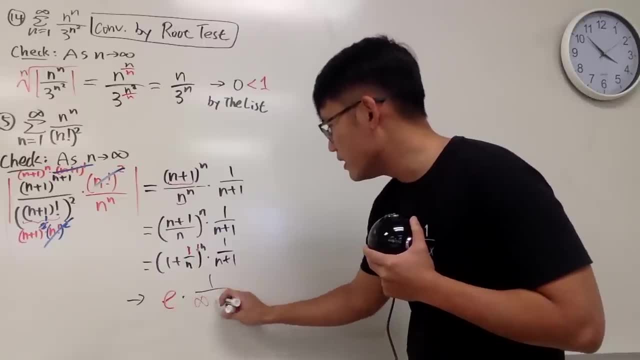 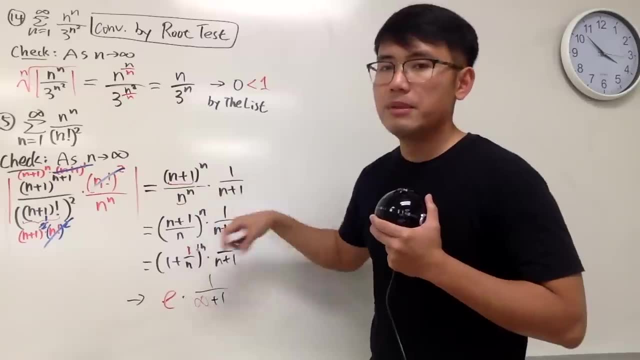 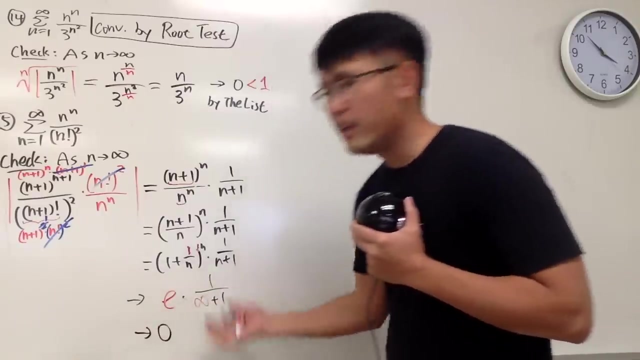 But this right here is 1 over infinity plus 1.. Remember the limit of a product. it's a product of a limit if both limits exist. This gives us e, this gives us 0.. So all in all, this right here is 0.. 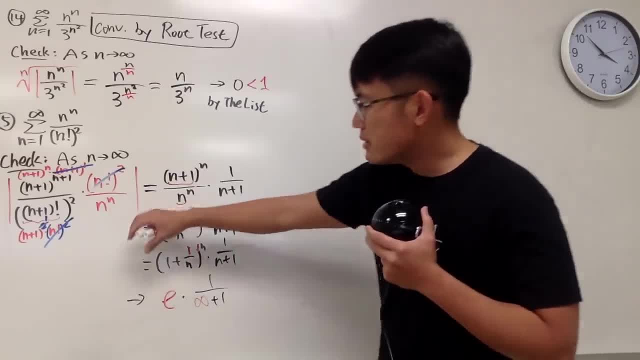 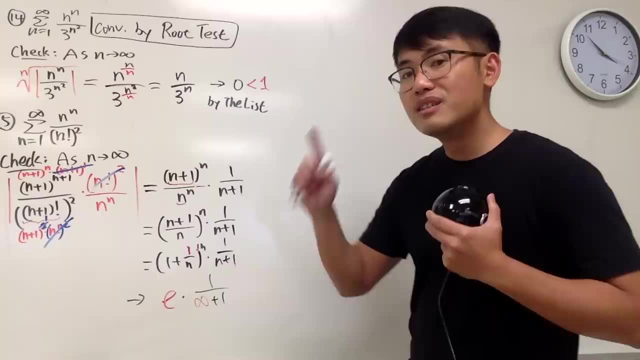 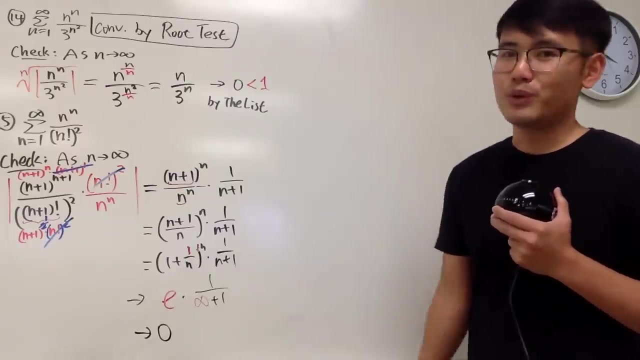 plus 1.. Remember, the limit of a product is a product of a limit if both limits exist. This gives us e. this gives us 0.. So all in all, this right here is 0.. So what can we do? right here. 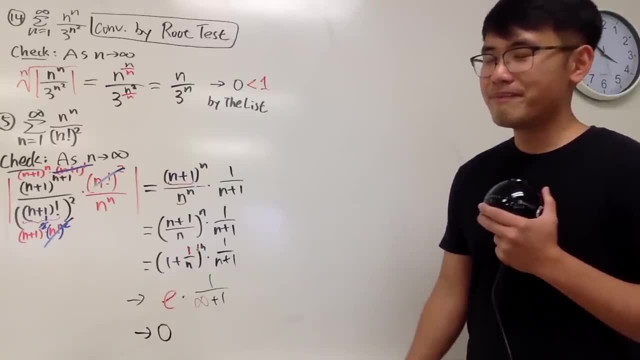 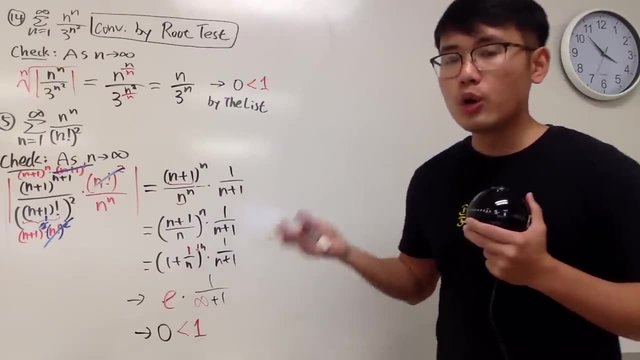 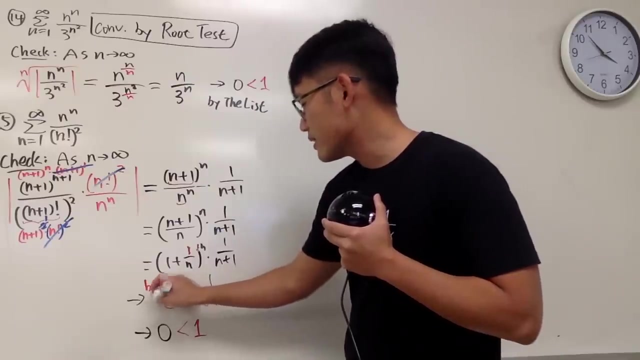 So what can we do? right here We can actually draw a conclusion. This right here is less than 1 from the ratio test, So we can actually draw a conclusion. So right here again, you can just say by the fact: 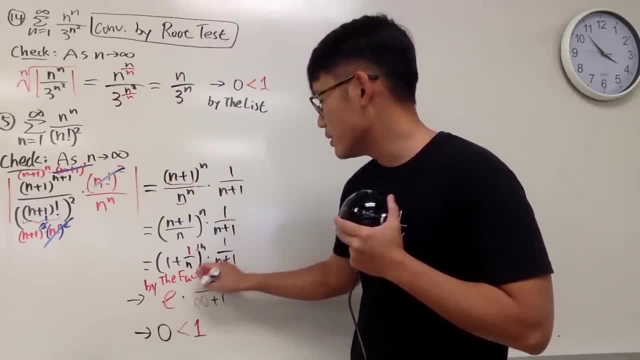 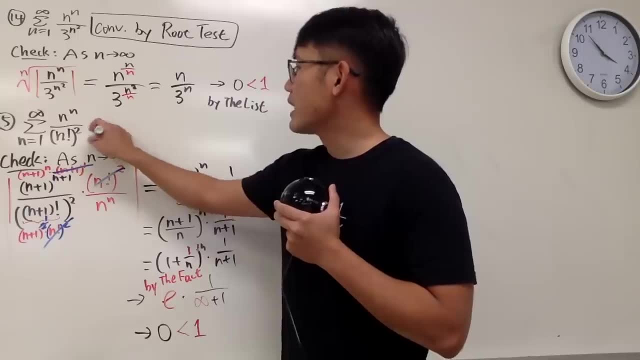 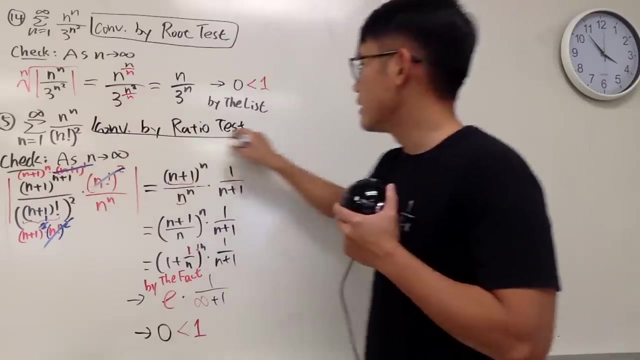 what the definition of e up to you. Just indicate that from here to here, right? Anyway, this is 0,, which is less than 1. So we can say this right here: converges by the ratio test, like that, right. 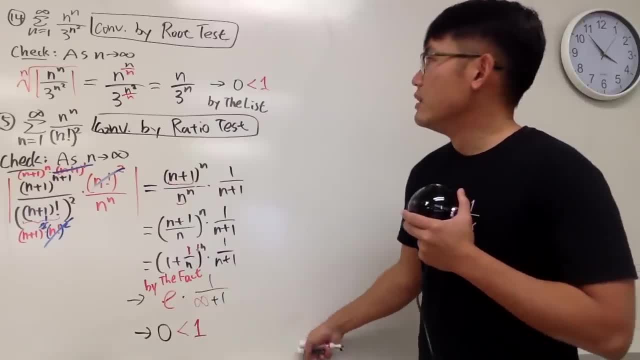 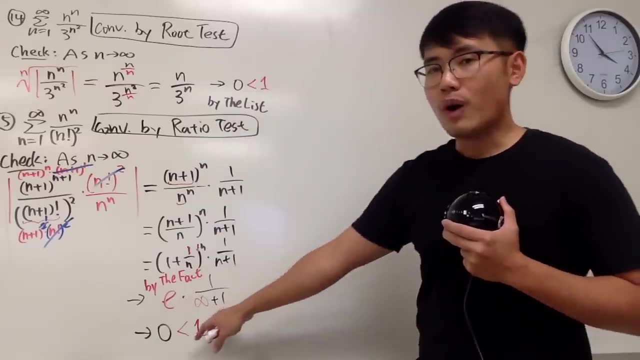 So that's very nice. Again for the ratio test and also for the root test. first, you cannot abbreviate them. Secondly, if you end up with 1 or 1 for the limits, we cannot draw any conclusion. We have to do more work for that right. 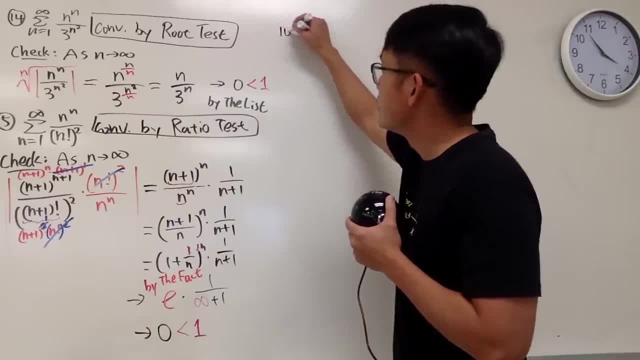 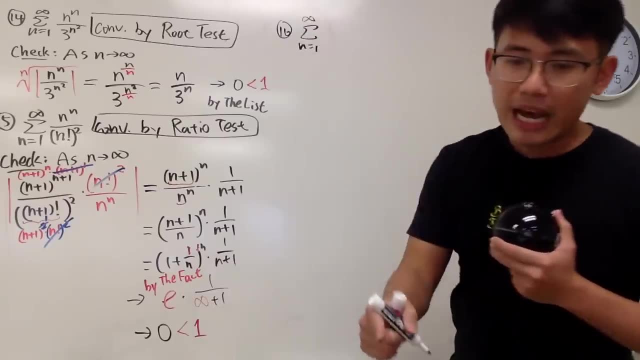 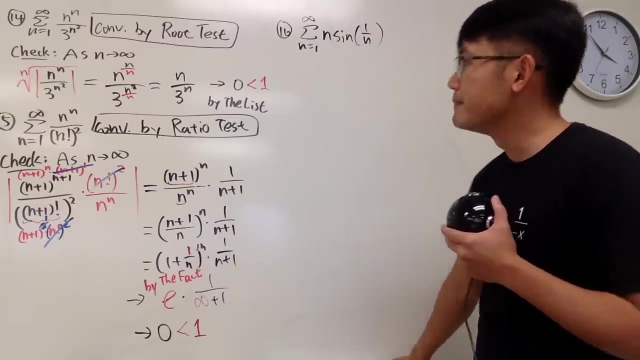 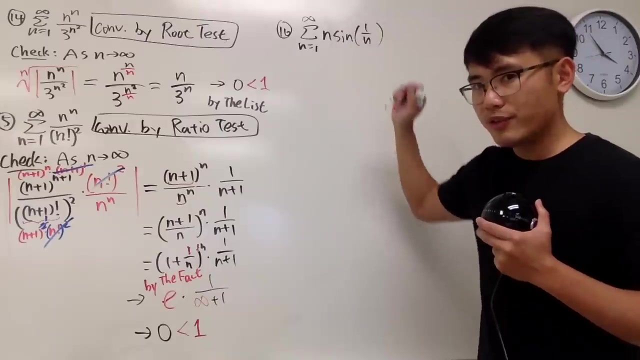 Okay, number 16, right here. Okay, the sum as n goes from 1 to infinity. And here we have n times sine of 1 over n. Check this out. If you just pay attention to this term, right, The a? n as n goes to infinity. 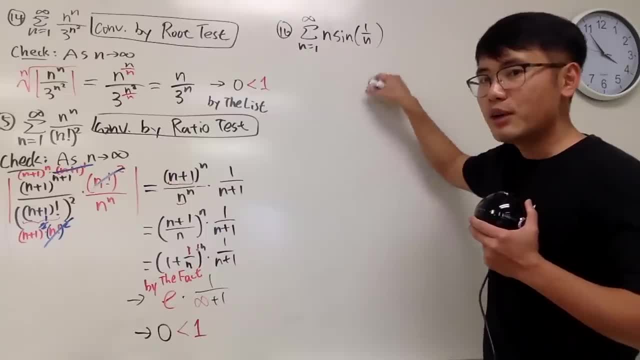 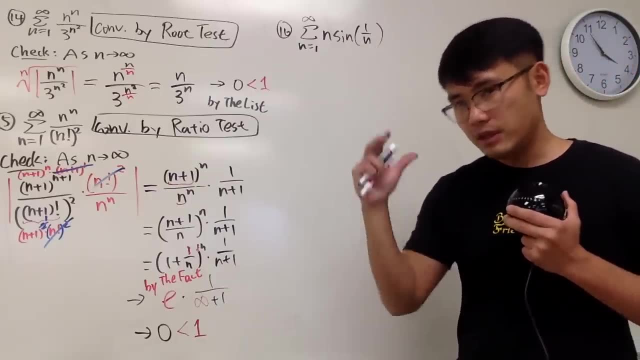 if you put infinity, here you get infinity times sine of 1 over infinity, which is 0. Sine of 0 is 0. In fact, here you end up with, in determinant form, infinity times 0. So what kind of you know? what answer do we get for the limit? 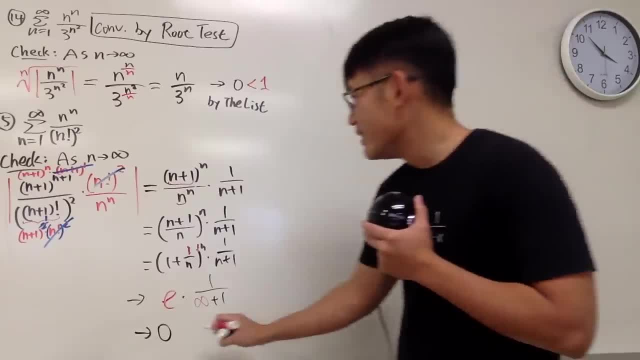 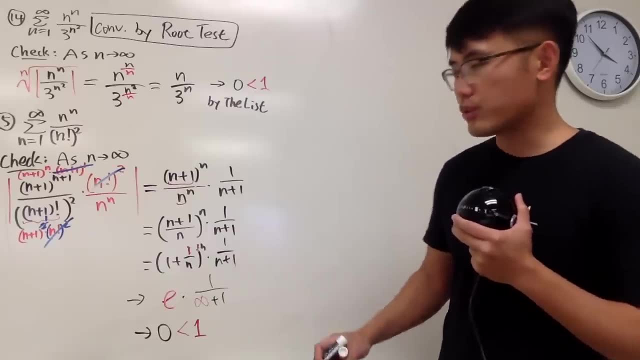 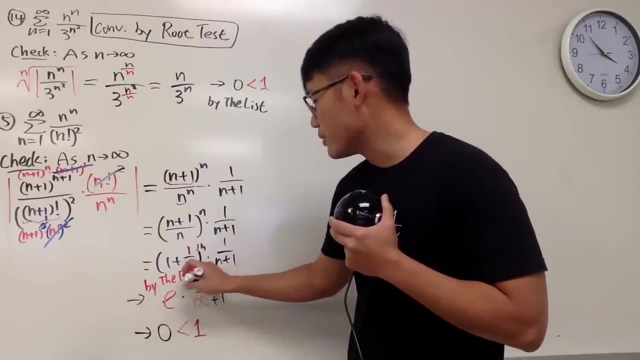 We can actually draw a conclusion. This, right here, is less than 1 from the ratio test, So we can actually draw a conclusion. So, right here again, you can just say by the fact what the definition of e up to you. 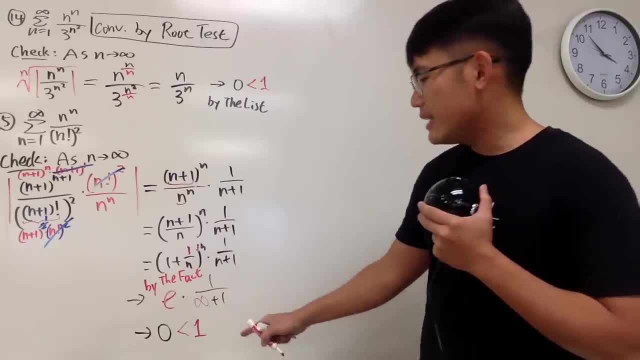 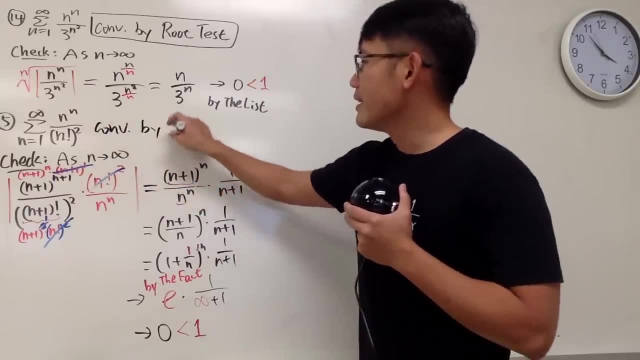 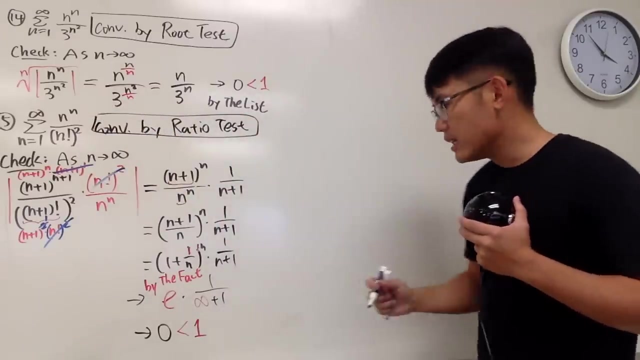 Just indicate that from here to here, right? Anyway, this is 0,, which is less than 1.. So we can say this right here: converges by the ratio test, Like that, right? So that's very nice Again. 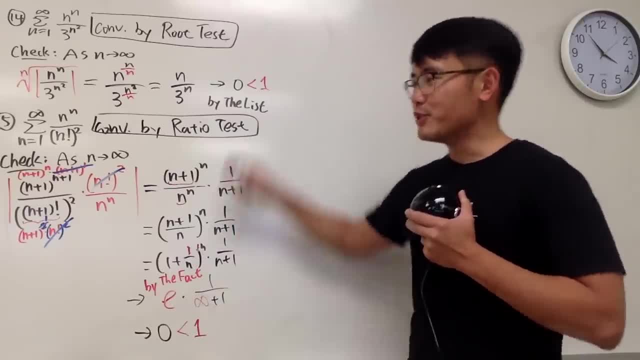 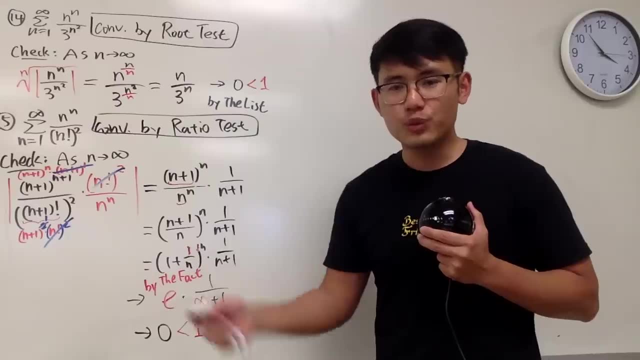 for the ratio test and also for the root test. first, you cannot abbreviate them. Secondly, if you end up with 1 over 1 for the limits, we cannot draw any conclusions. We have to do more work for that Right. 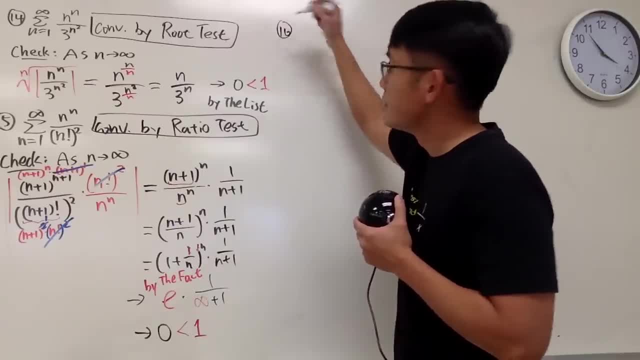 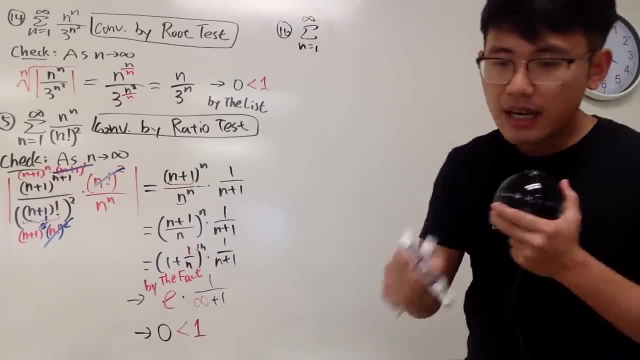 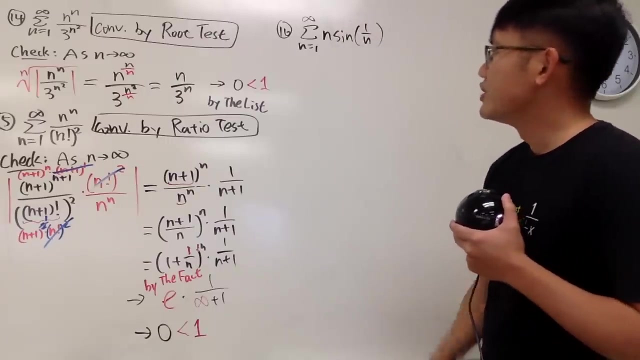 Okay, number 16 right here. Okay, the sum as n goes from 1 to infinity, And here we have n times sine of 1 over n. Hmm, Check this out, If you just pay attention to this term, right, The? 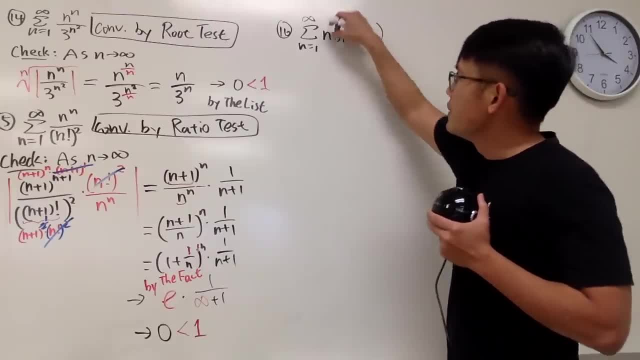 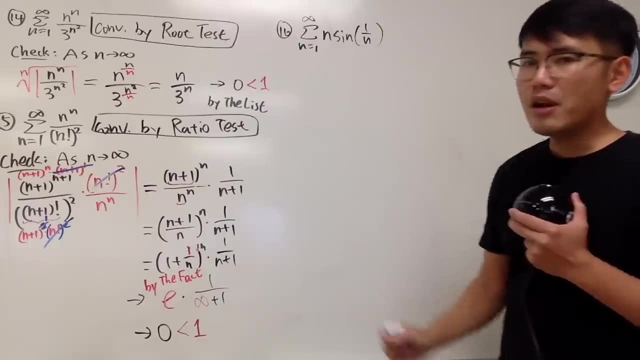 a n As n goes to infinity. if you put infinity here, you get infinity times sine of 1 over infinity, which is 0. Sine of 0 is 0. In fact, here you end up with, in determinant form, infinity. 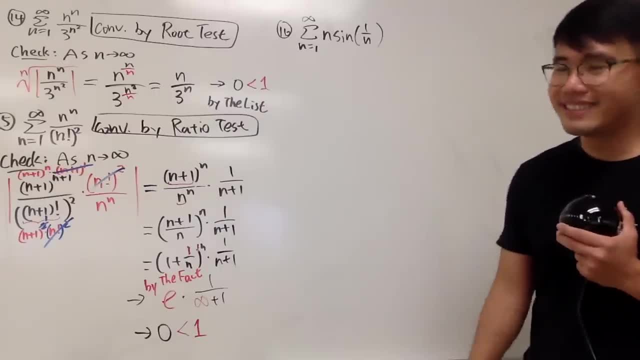 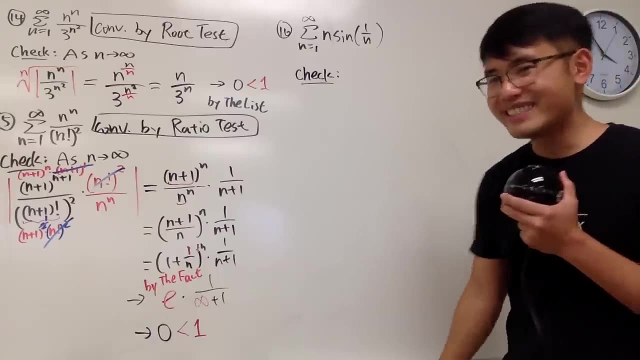 times 0.. So what kind of you know what answer do we get for the limit? Well, we are going to just check the limit. This is the limit test or the test for divergence. So let's do that, So we'll just take. 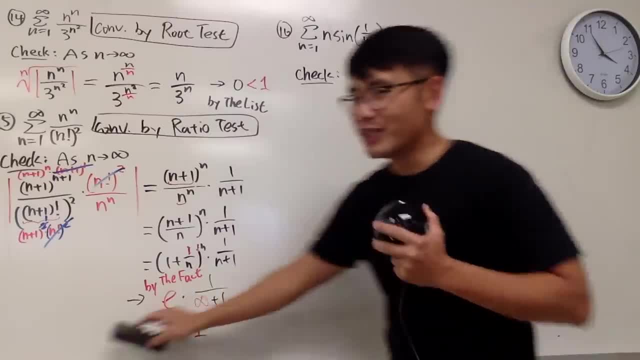 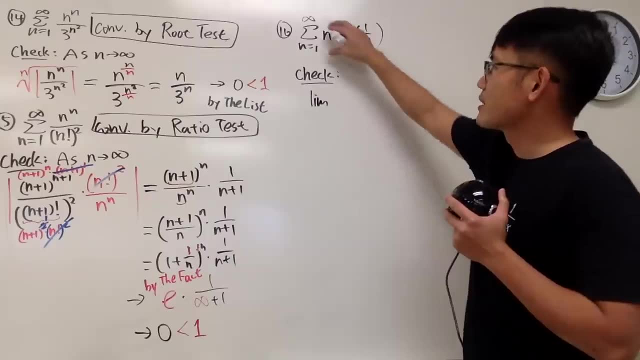 I think for the test for divergence I will really just write down the LIM to make it specific, because one of the common mistakes is that people get confused with the sum and also the LIM notation. So let me just really write this down. 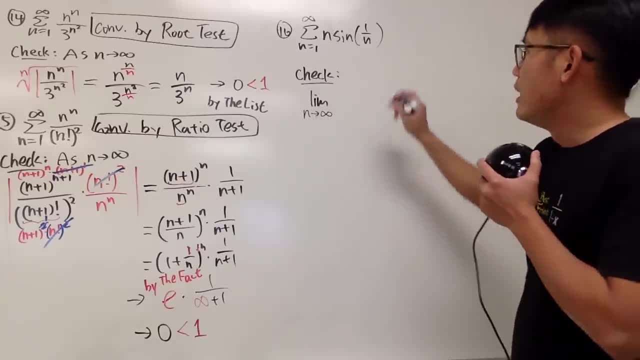 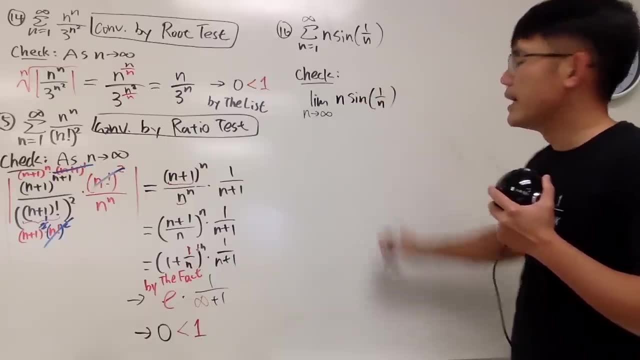 We'll just check the limit, as n goes to infinity Of this term. right Of this a n thing. So it's just n times sine of 1 over n, like this. Hmm, We do have an infinity times 0 situation. 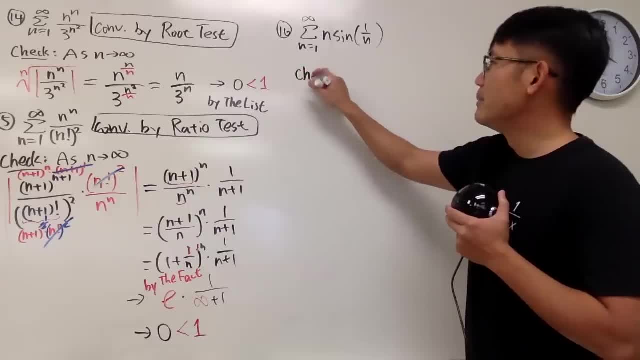 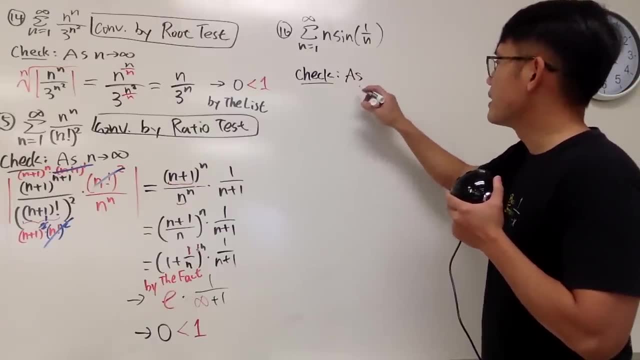 Well, we are going to just check the limit. This is the limit test or the test for divergence. So let's do that, So we'll just take, I think, for the test for divergence. I will really just write down the LIM. 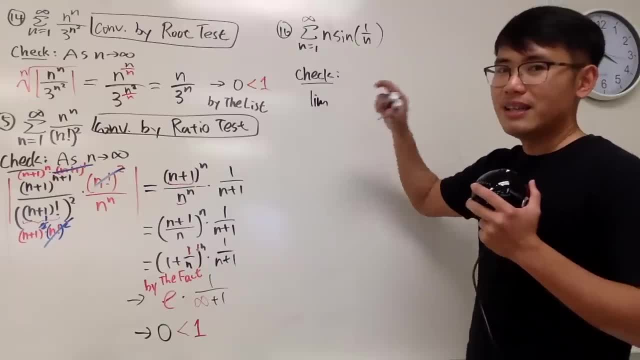 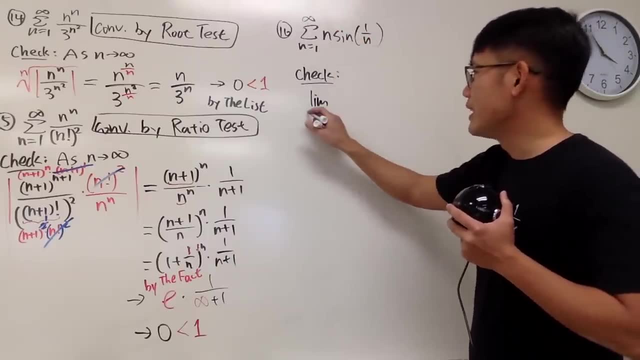 to make it specific, because one of the common mistakes is that people get confused with the sum and also the LIM notation. So let me just really write this down. We'll just check the limit, as n goes to infinity of this term, right? 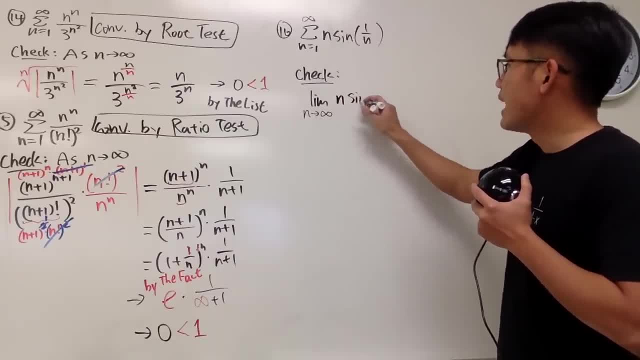 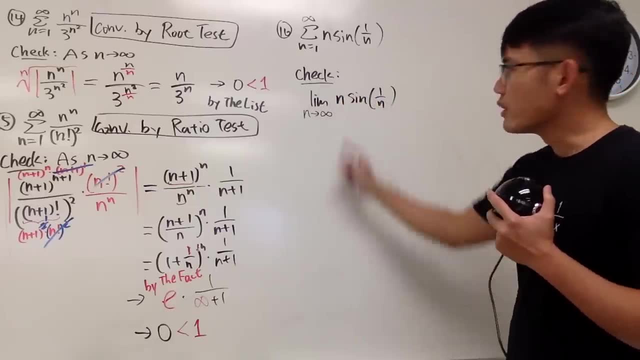 Of this a n thing. So it's just n times sine of 1 over n, like this. Hmm, We do have an infinity times 0 situation, So let me bring the n down down. In another word we will end up with: 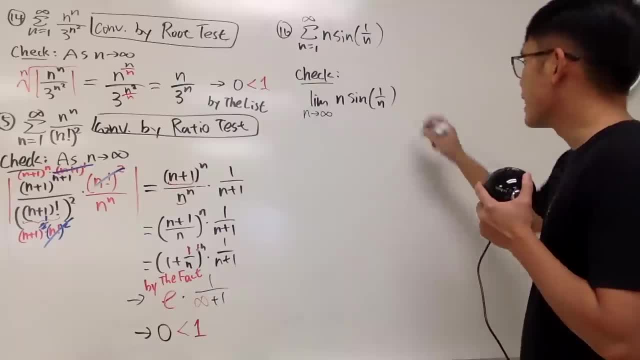 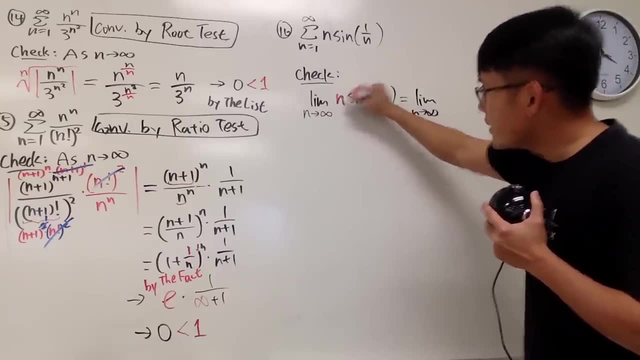 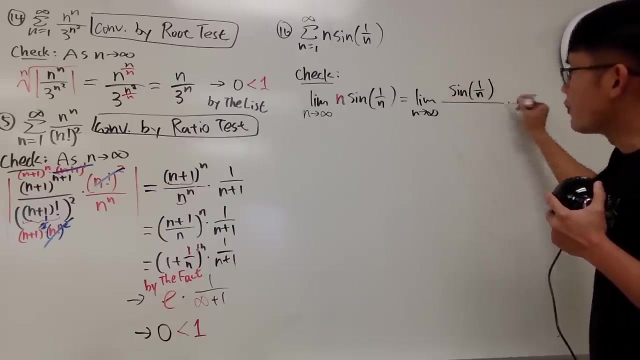 So let me bring the n down down. In another word, we will end up the limit as n goes to infinity. If you look at this n right here, well, we end up with sine of 1 over n. over that, down, down becomes. 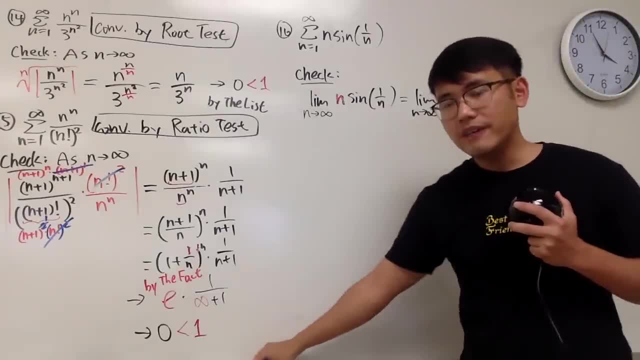 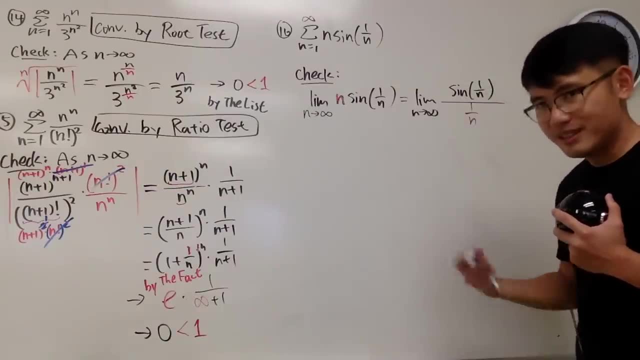 1 over n like this, And here, in fact, you can do a few things. Notice, if n goes to infinity, this is approaching 0.. That's also approaching 0. So, technically, you can do the following And you have. 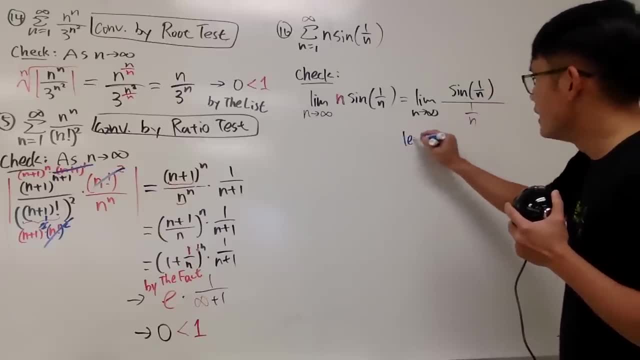 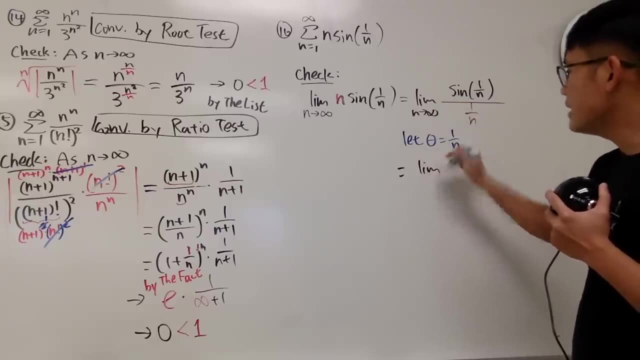 to make sure they are the same right. So I will just say that theta equals 1 over n, And now, as n goes to infinity, we'll see that this is the limit as theta goes to infinity. to here you get. theta is approaching 0.. 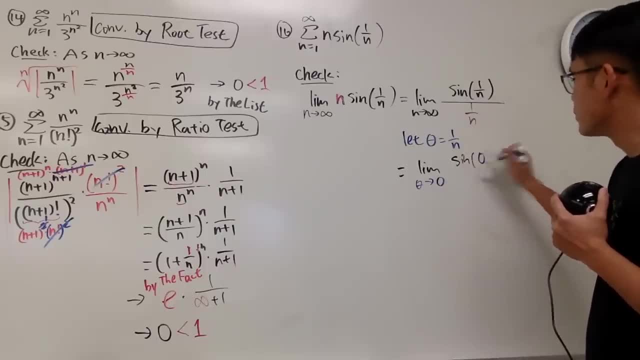 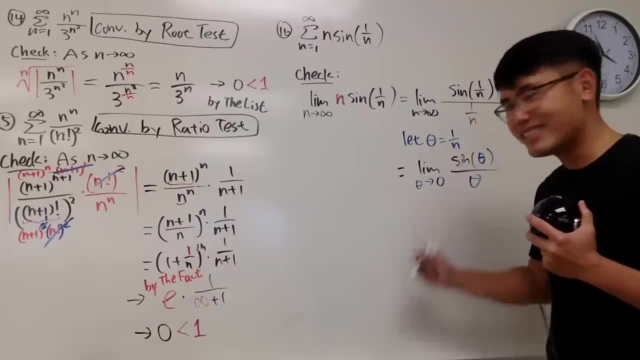 And of course we end up with sine of 0. I mean sine of theta. And then here is also theta. What's this? This right here is the limit. This right here is equal to 1.. And I'll just tell you guys. 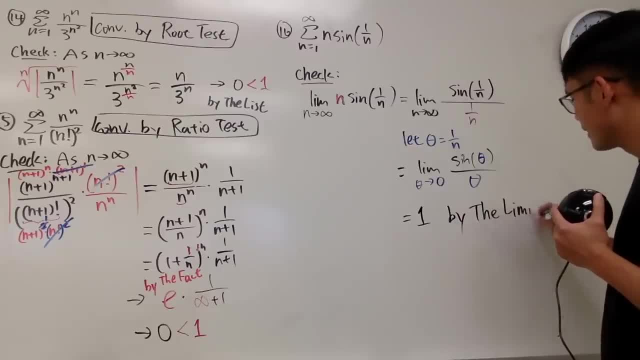 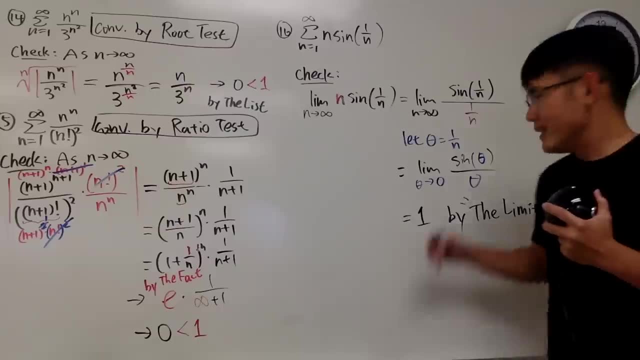 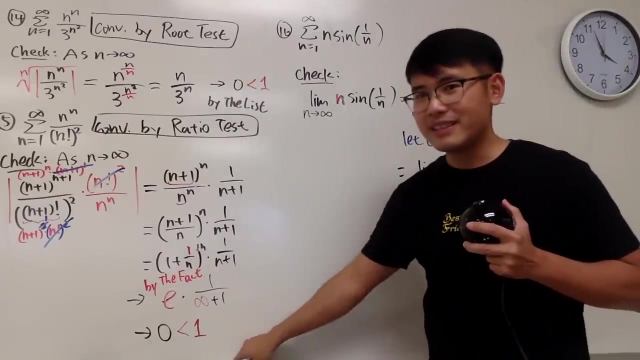 by the limit Right And right here. please do not do Lapithov's rule Seriously. If you see this, yes, you can put down 1. But don't say Lapithov's rule, right, That's like the most. 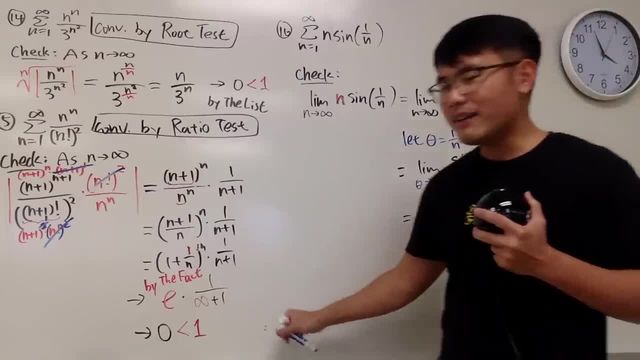 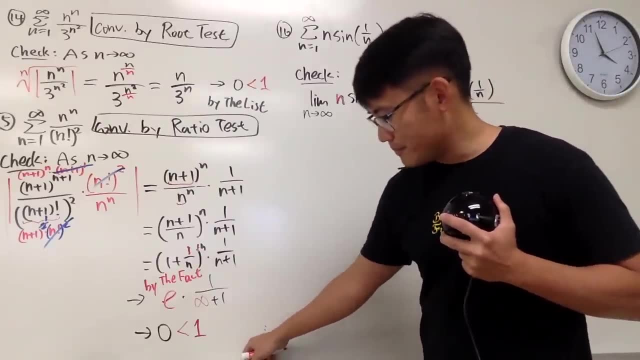 confusing limit Like: why not? I have a video on that. To be honest, that video is not good enough, so I will make another one. But I know some people will tell me to comment why we don't use Lapithov's. 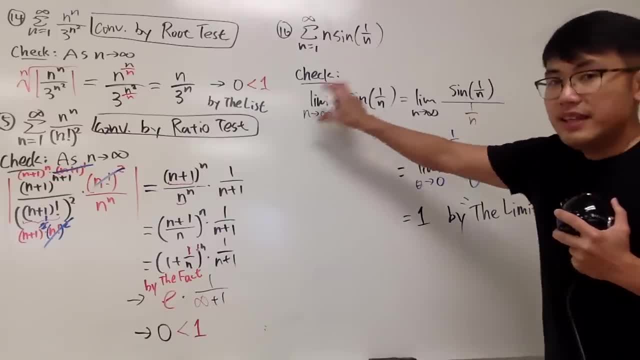 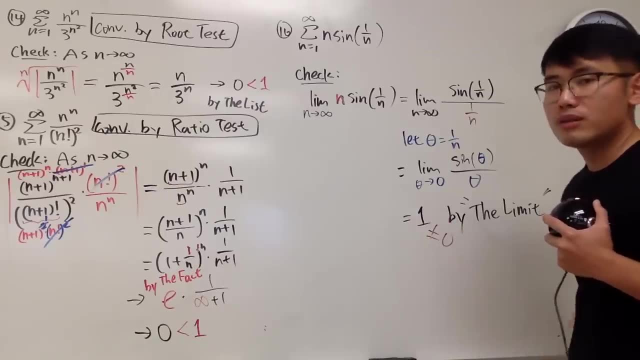 rule, so tell me to do so as well. Anyway, this limit. blah, blah blah, we get 1.. And you have to know that 1 is not the same as 0.. Huh, Look at all these confusing numbers. You have to be really. 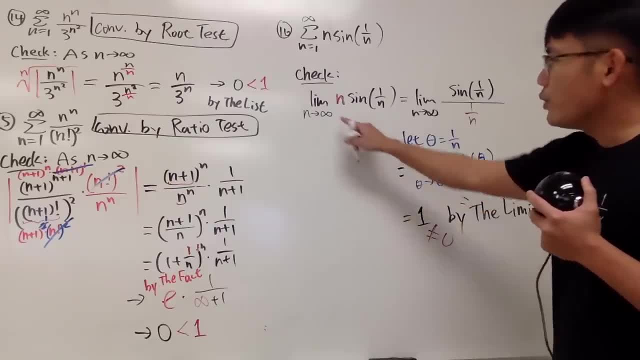 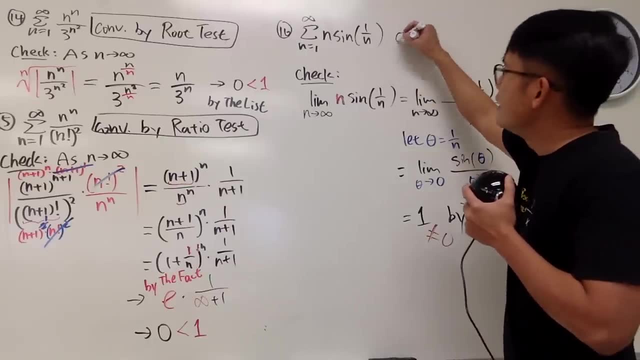 you have to think really carefully of all this When you are doing the limit test, the test for divergence. if you don't end up with 0, game over, You can come back here and say this right here: Divergence by. 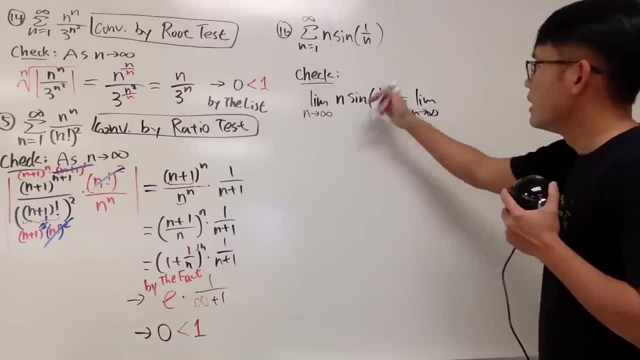 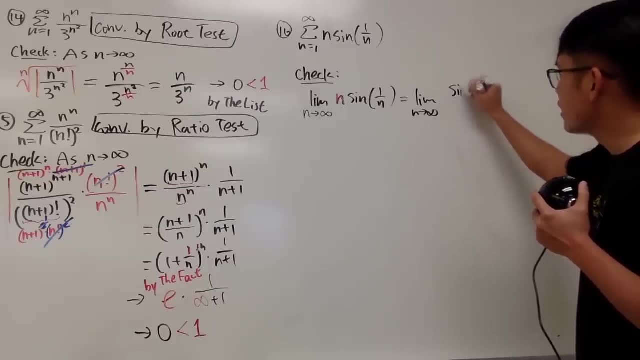 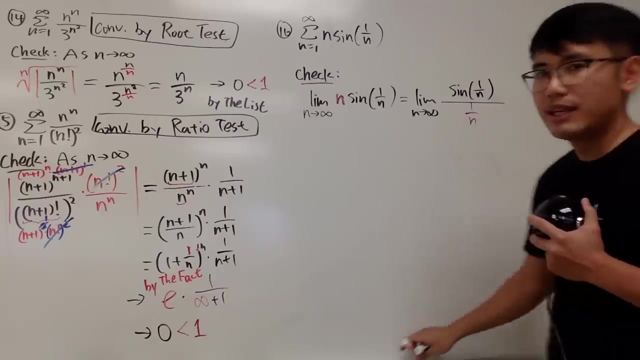 we will end up the limit as n goes to infinity. If you look at this n right here, well, we end up with sine of 1 over n. over that down, down becomes 1 over n, like this, And here, in fact, you can do a few things. 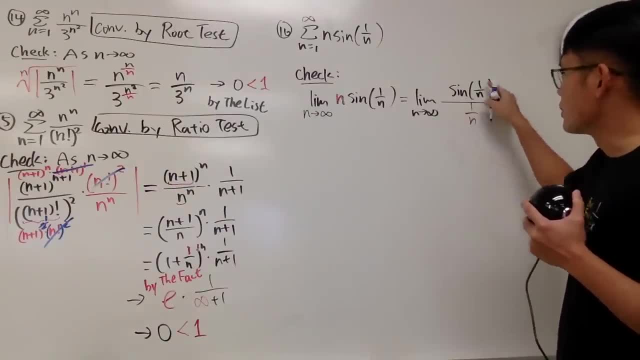 Notice: if n goes to infinity, this is approaching 0.. That's also approaching 0. So technically you can do the following And you have to make sure they are the same right. So I will just say that theta equals 1 over n. 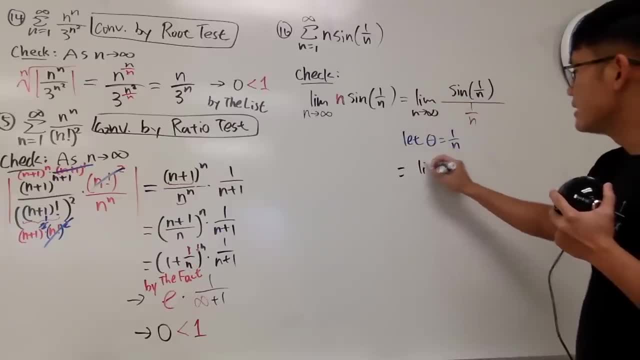 And now, as n goes to infinity, we'll see that this is the limit. as theta goes to infinity, to here You get: theta is approaching 0.. And of course, we end up with sine of 0, I mean sine of theta. 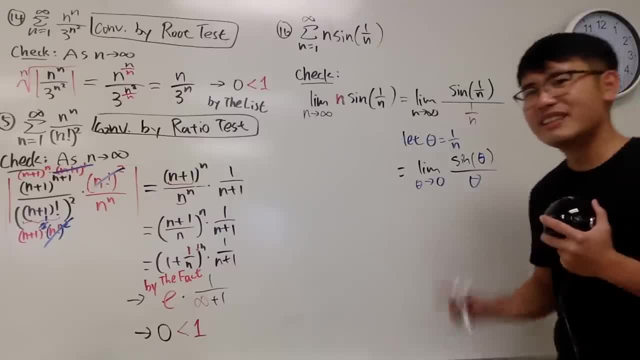 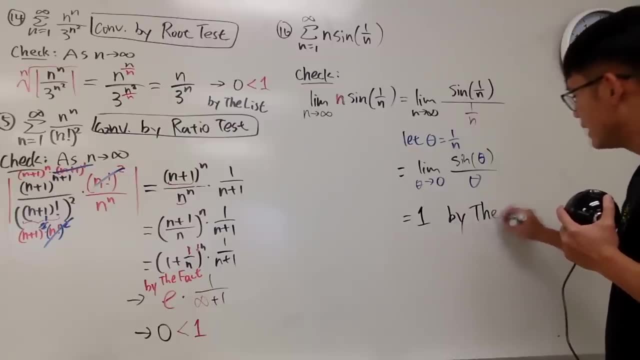 And then here is also theta. What's this? This right here is the limit, This right here is equal to 1.. And I'll just tell you guys, by the limit, right And right here, please do not do Lapito's rule. 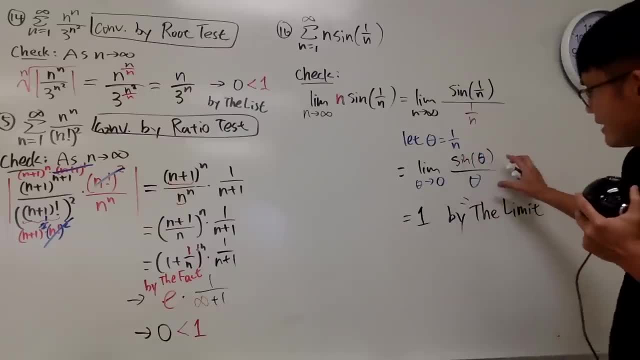 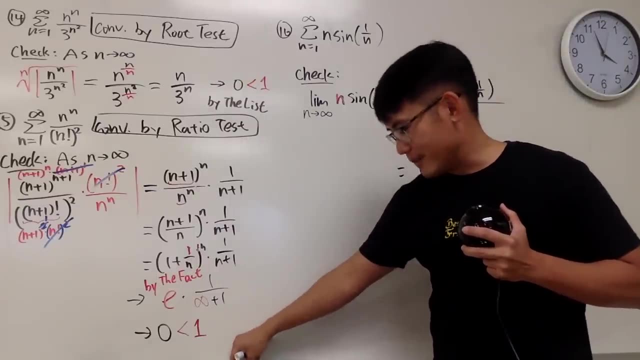 Seriously, if you see this, yes, you can put down 1, but don't say Lapito's rule, right? That's like the most confusing limit, Like why not? I have a video on that. To be honest, that video is not good enough. 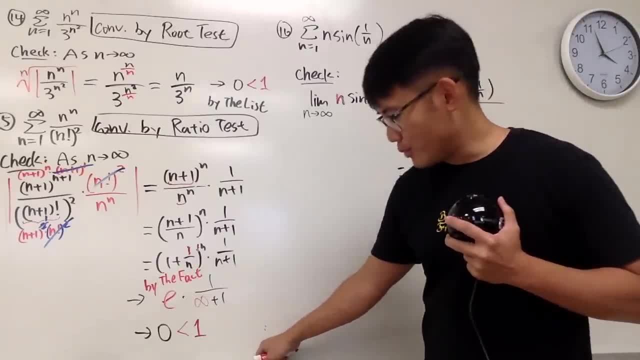 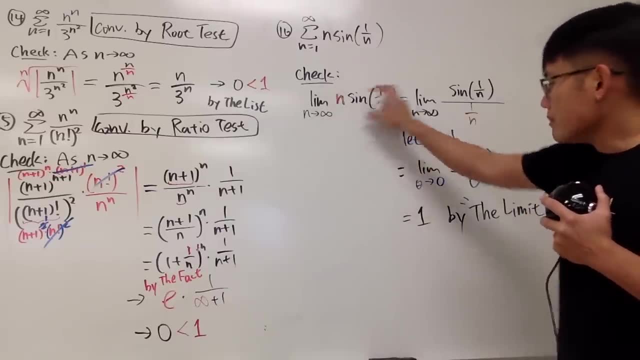 so I will make another one. But I know some people will tell me to comment why we don't use Lapito's rule, so tell me to do so as well. Anyway, this limit, blah, blah, blah, we get 1.. 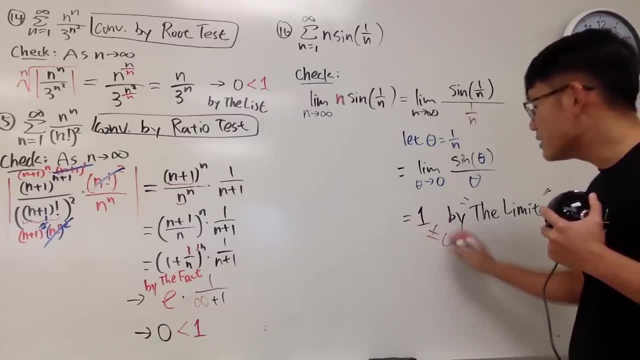 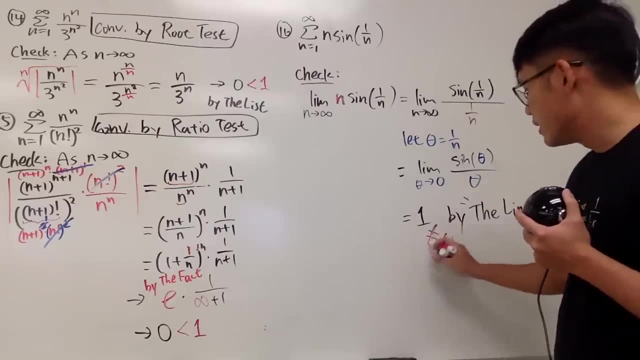 And you have to know that 1 is not the same as 0. Huh, look at all these confusing numbers. You have to be really, you have to think really carefully of all this When you are doing the limit test, the test for divergence. 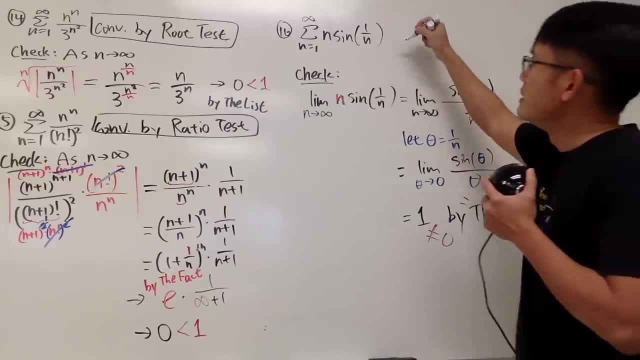 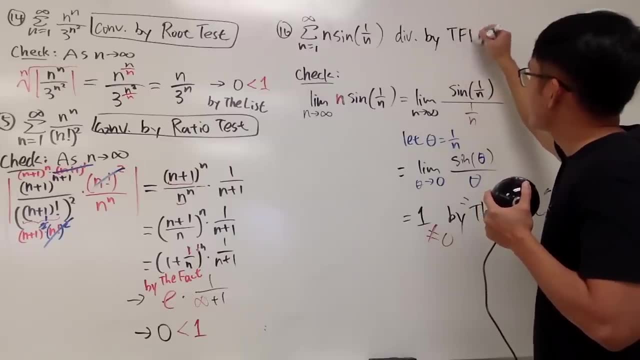 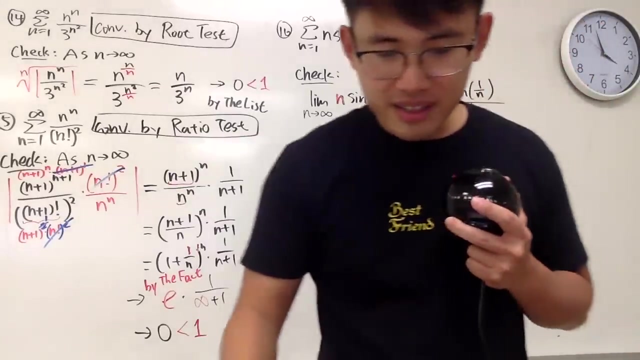 if you don't end up with 0, game over, You can come back here and say this right here: Divergence By the test for divergence. Okay, So that's it. That's the best situation ever. Okay, now we will continue. 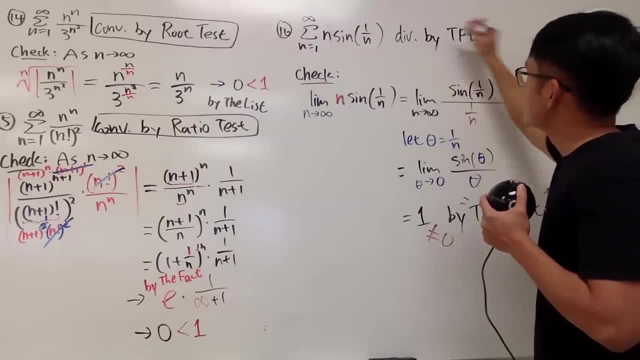 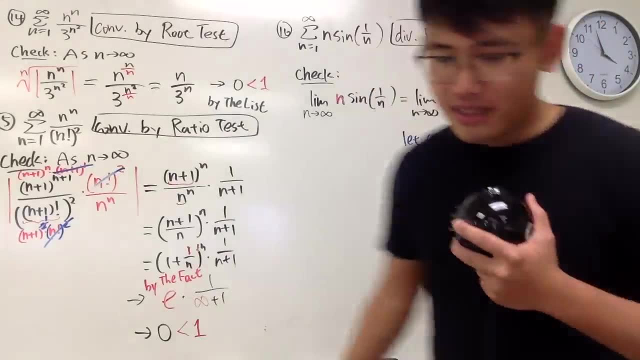 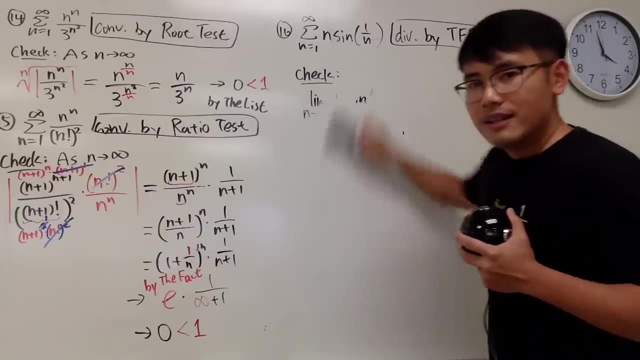 the test for divergence. Okay, So that's it. That's the best situation ever. Okay, now we will continue Seriously, if you guys are still watching. well, you're working hard and thank you guys, so much It's been. 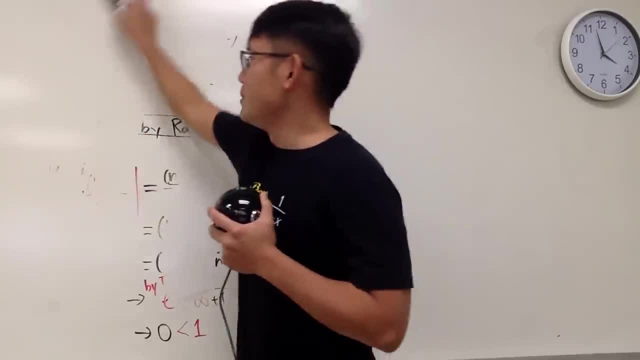 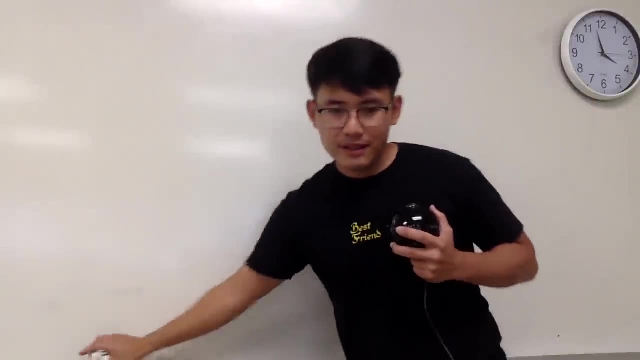 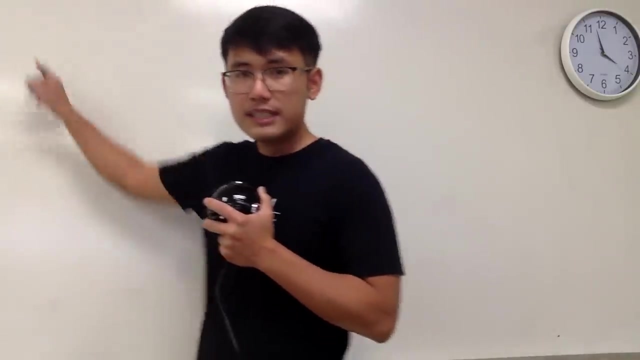 1 hour and 30 minutes, and if you are still watching, just give me a time stamp. You guys know the deal. Okay, so now that was number 16, and we'll move on to number 17 right here. So here we go. 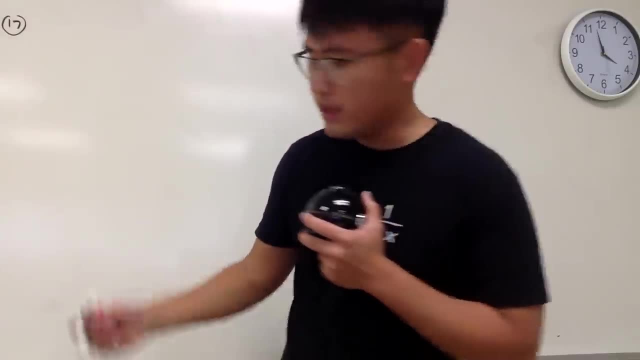 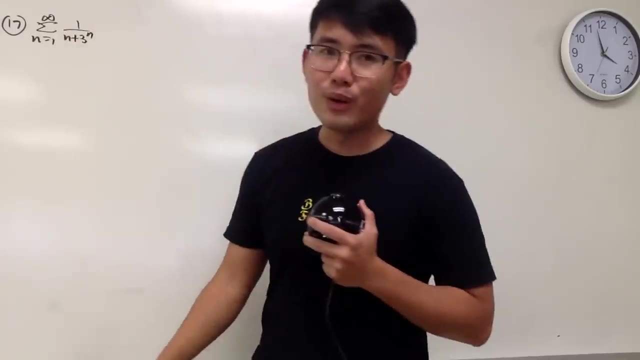 number 17.. We have to deal with this. The sum as n goes from 1 to infinity, 1 over n plus 3 to the nth power. By now, this right here should be pretty easy. This right here. I'll just put a note. 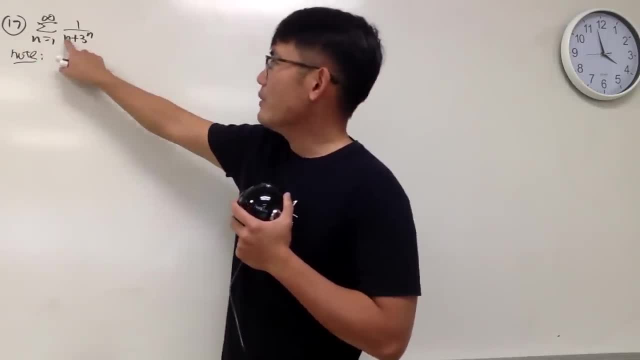 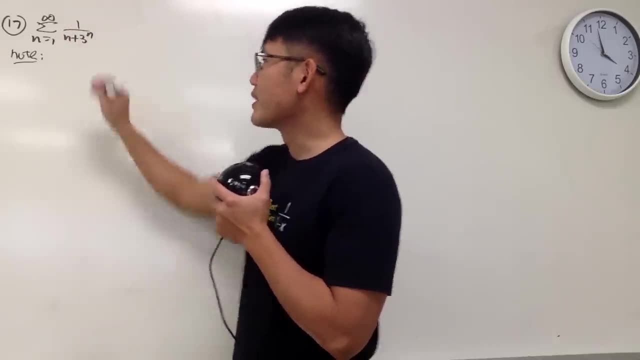 right here for you guys. Well, you're adding n. If you ignore that, it will be less than n. 1 over 3 to the n is geometric, so you can just draw a conclusion real quick. So here we go. This is the sum. 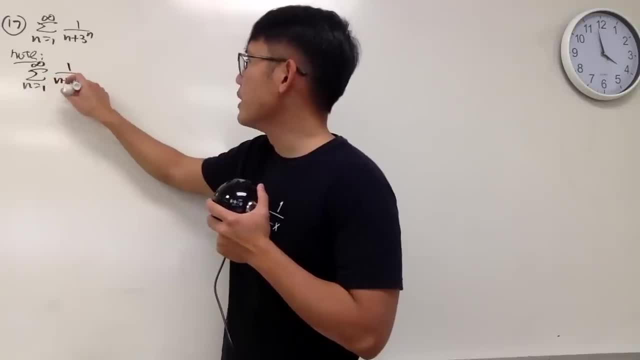 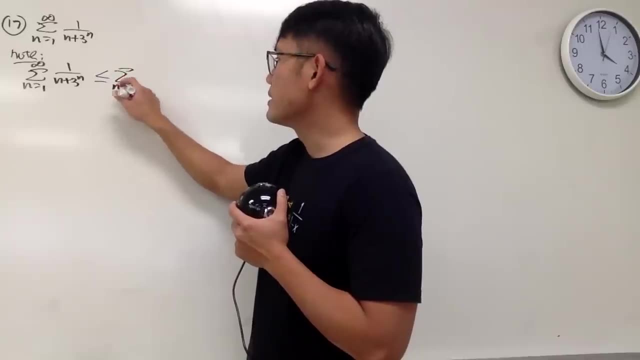 as n goes from 1 to infinity, 1 over n plus 3 to the nth power. Just take the n out and we will get less than or equal to the sum, as n goes from 1 to infinity, 1 over 3 to the nth. 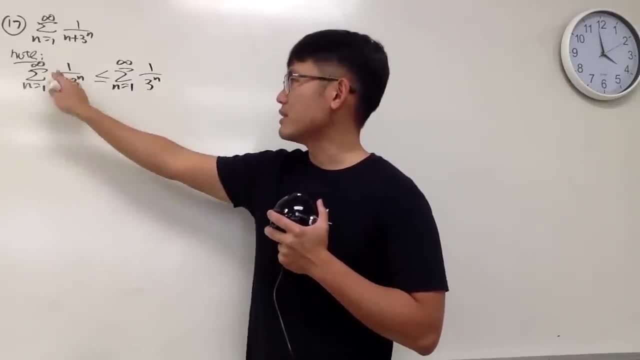 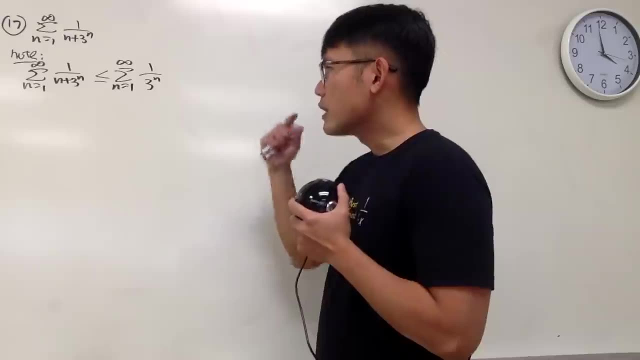 power. right, Because again, n is positive, so get that out. That's good. The bigger the denominator, the smaller the fraction is just like that. So that's pretty much the idea and right here of course you can see. 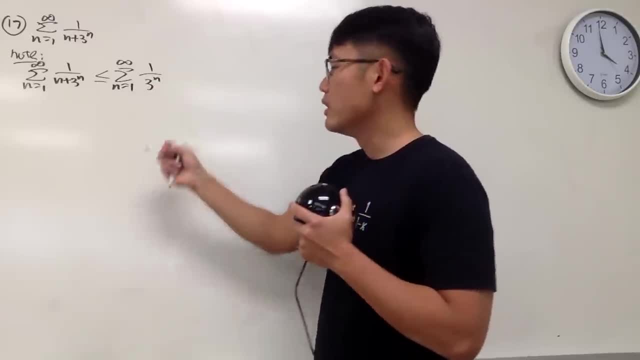 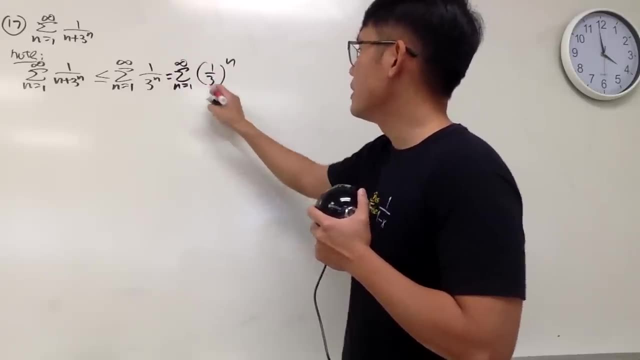 this is 1 over 3 and n to the nth power. so you can just indicate that this is the sum, as n goes from 1 to infinity, 1 over 3 to the nth power, and here r is equal to 1 over 3, and. 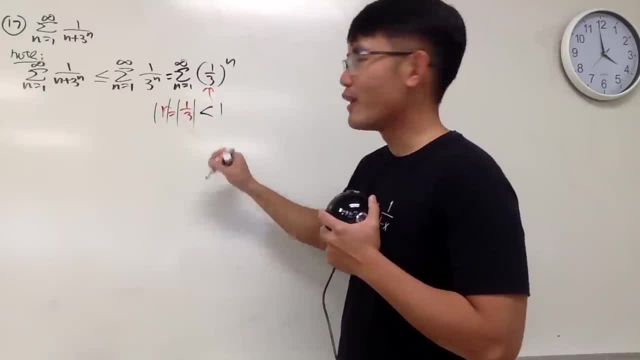 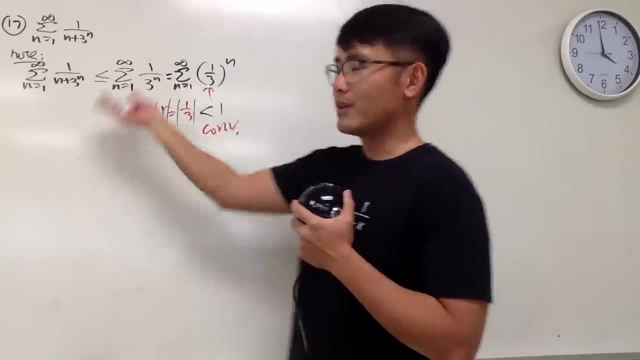 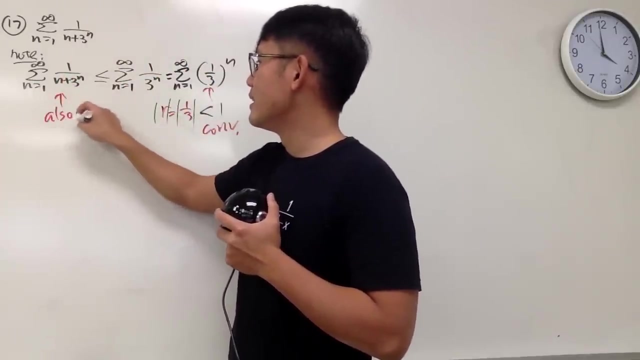 if you take the absolute value of the r, which is less than 1, this right here, converges by geometric series. So we will- well, I cannot say this converges by geometric. I will have to say this right here also converges right And 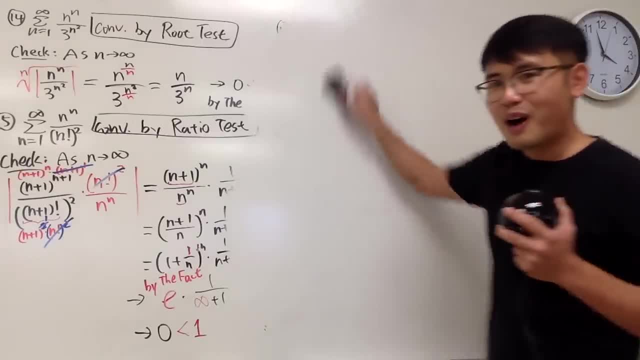 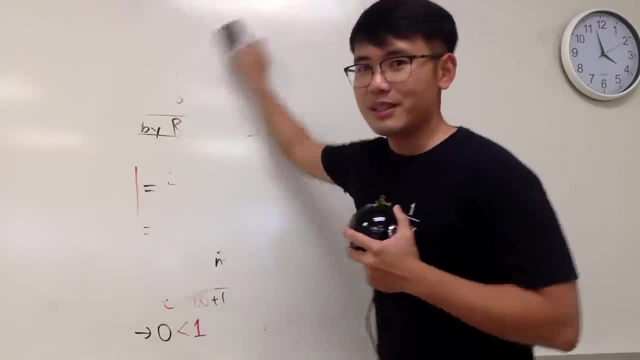 Seriously, if you guys are still watching, well, you're working hard and thank you guys. so much. It's been 1 hour and 30 minutes And if you are still watching, just give me a time stamp. You guys know the deal. 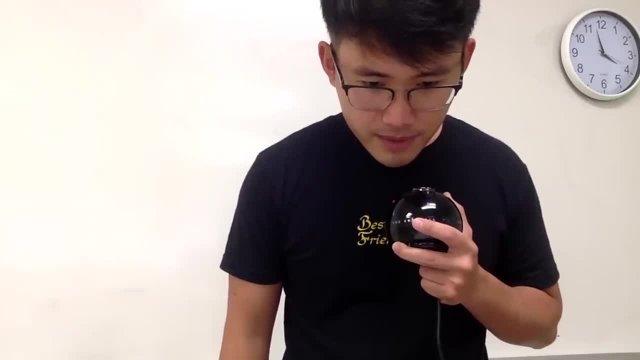 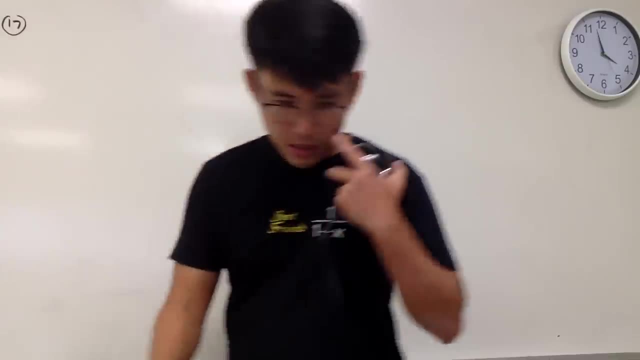 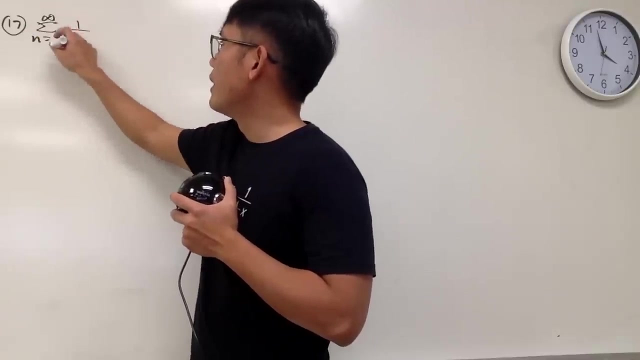 Okay, so now that was number 16, and we'll move on to number 17 right here. So here we go, number 17.. We have to deal with this. the sum as n goes from 1 to infinity, 1 over n plus 3 to the nth power. 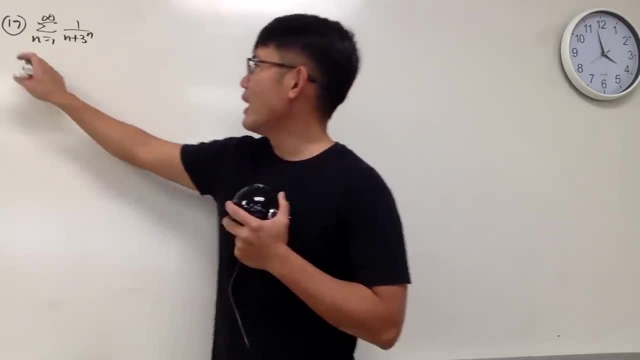 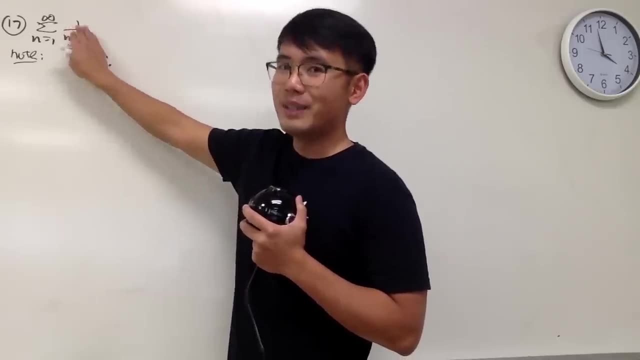 By now. this right here should be pretty easy, This right here. I'll just put a note right here for you guys. Well, you're adding n. If you ignore that, it will be less than n. 1 over 3 to the nth is geometric. 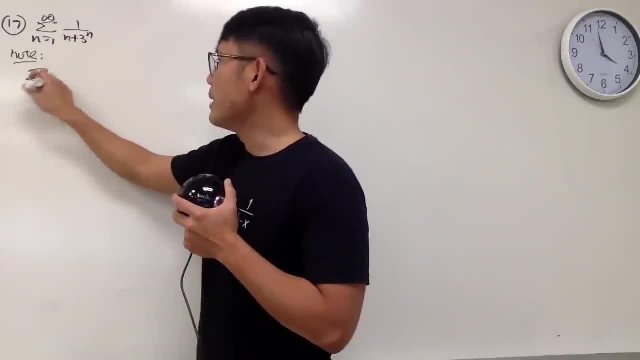 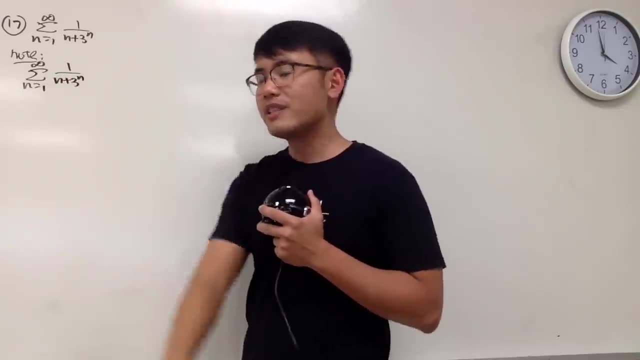 so you can just draw a conclusion real quick. So here we go. This is the sum as n goes from 1 to infinity, 1 over n, plus 3 to the nth power. Just take the n out and we will get less than or equal to. 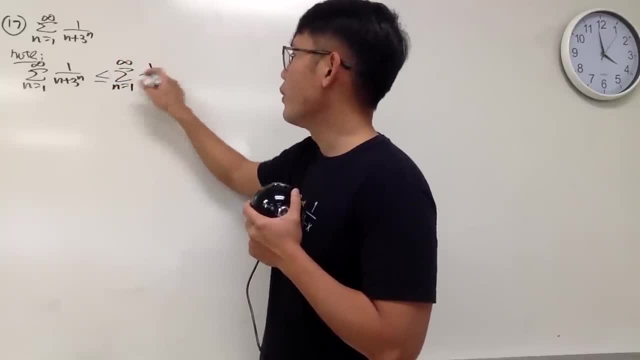 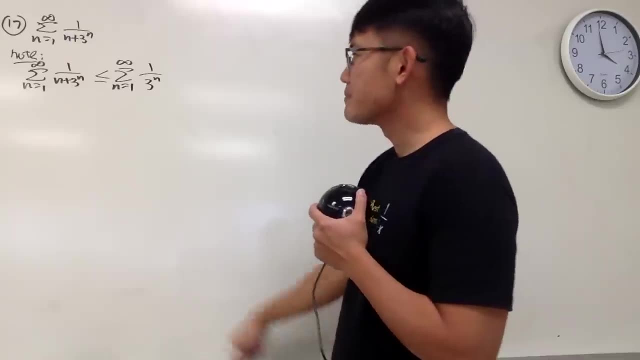 the sum as n goes from 1 to infinity, 1 over 3 to the nth power. Right, Because again n is positive. so get that out, That's good. Bigger the denominator, the smaller the fraction is just like that. 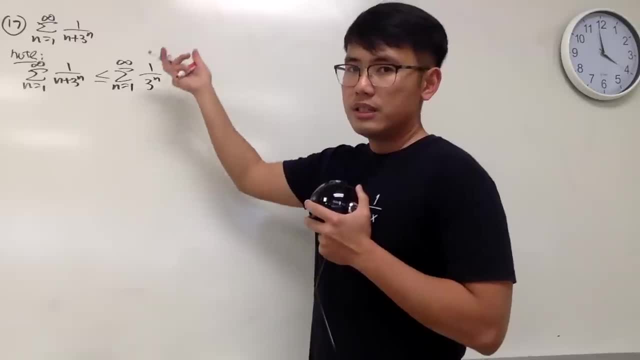 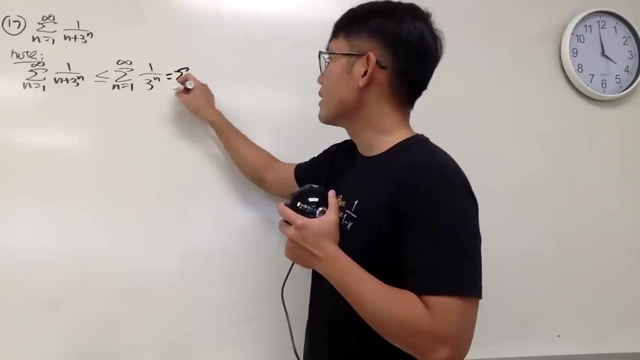 So that's pretty much the idea, and right here of course you can see this is 1 over 3 and then to the nth power. so you can just indicate that this is the sum as n goes from 1 to infinity. 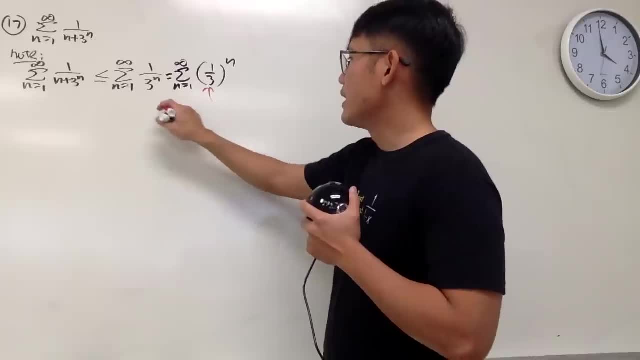 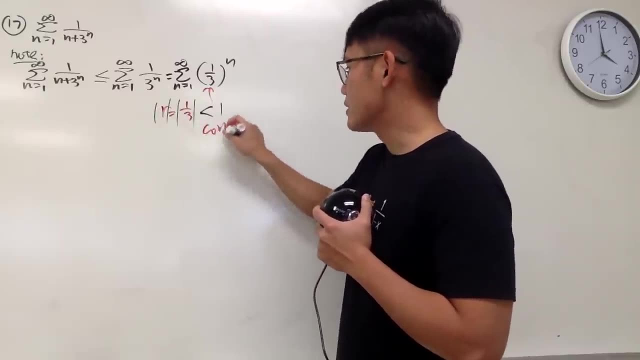 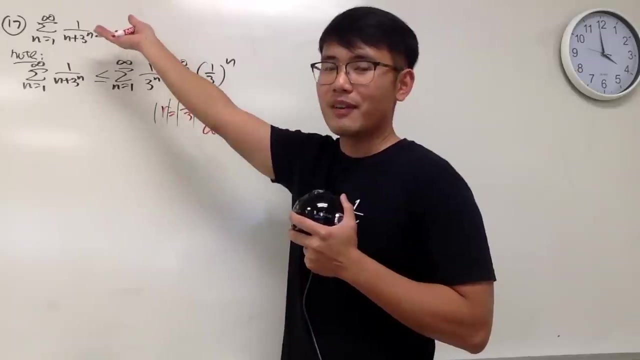 1 third, nth power, and here r is equal to 1 third. and if you take the absolute value of the r, which is less than 1, this, right here, converges by geometry series. So we will- well, I cannot say this: converges by geometry. 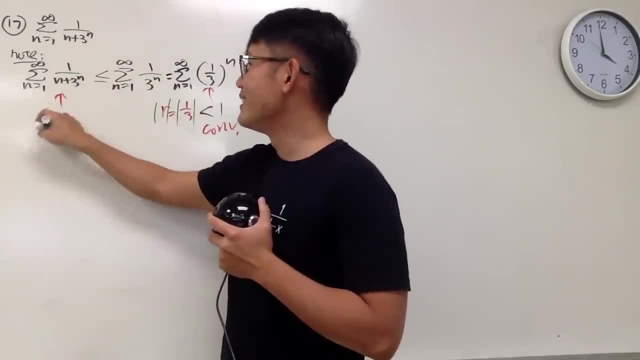 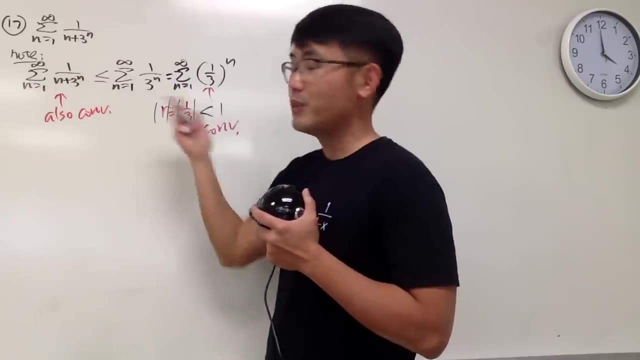 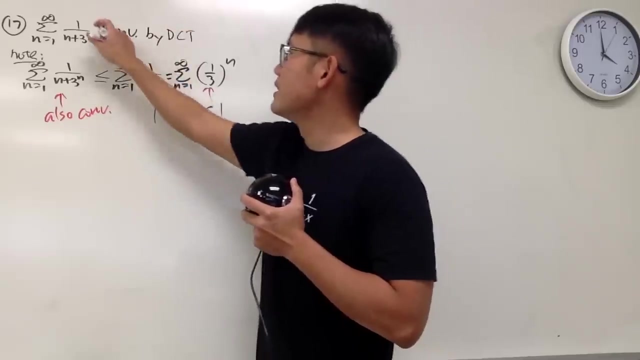 I will have to say this right here also: converges right, And the reason I will say this is also convergence because we did the comparison. So I will just come back here and say this right here: converges by direct comparison test. Oh man, I wish every question is this. 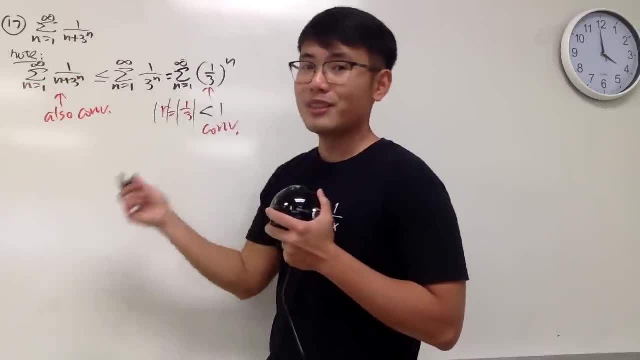 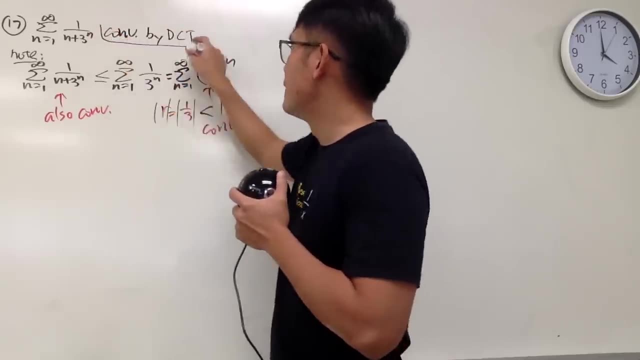 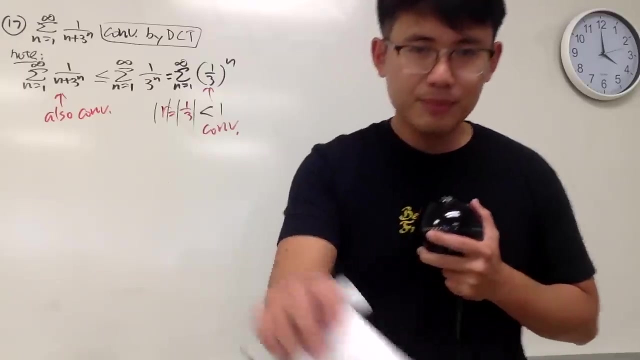 the reason that we say this is also convergent is because we did the computer set, So I will just come back here and say this right here: converges by direct comparison test. Oh man, I wish every question is that easy, Number 18.. 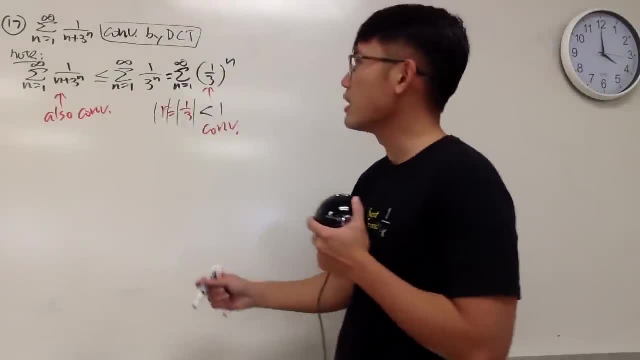 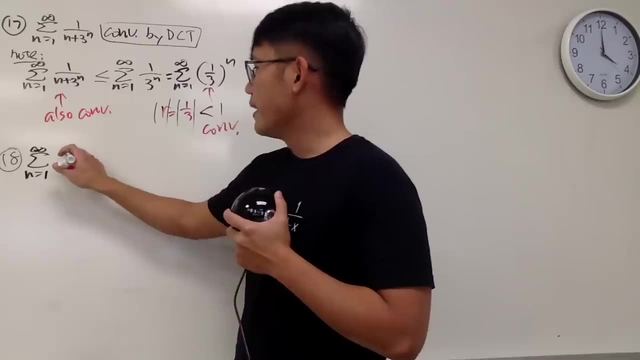 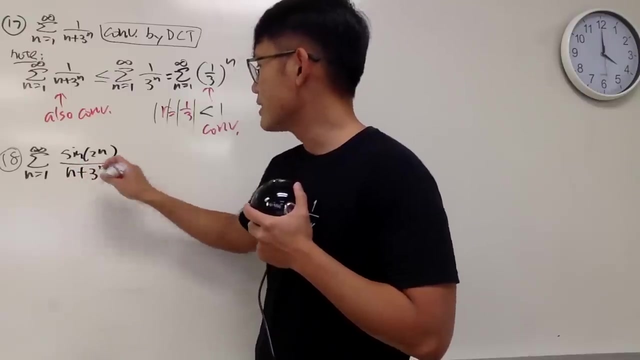 Very similar, God. should I see number 18.. We are going to do the sum as n goes from 1 to infinity, sine of 2n over and bottom. here we have n plus 3 to the nth power, like that. Remember what I told you guys earlier. 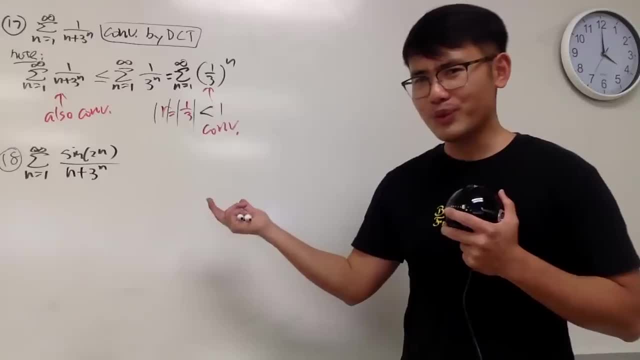 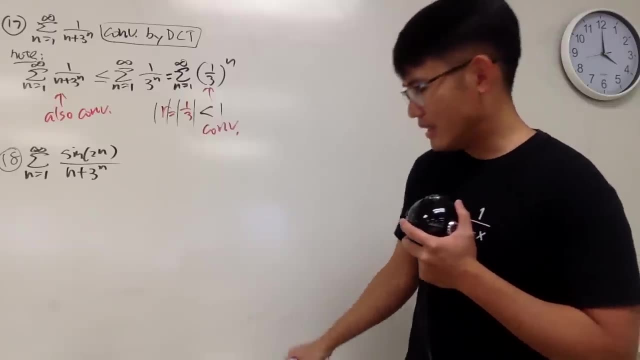 When we see sine cosine in this kind of situations, what do we do? Take the absolute value. Sometimes, sine cosines, they cannot make up their minds. They will be negative sometimes. Don't let the negatives bother you. I will keep that in mind myself. 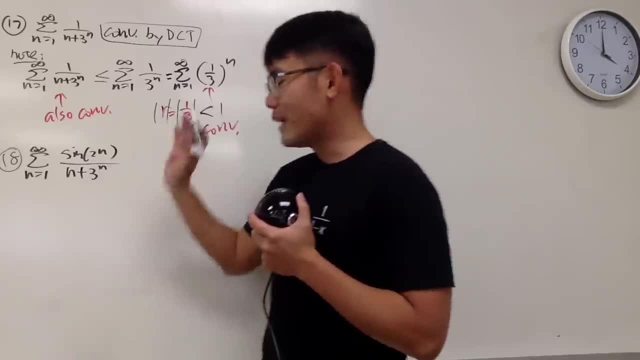 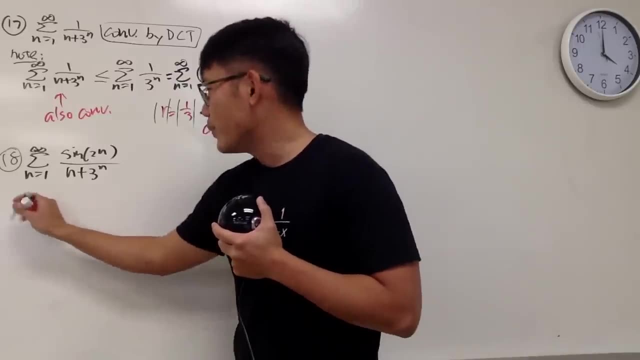 as well, because I do have haters. you guys don't know that, So I will keep that in mind. if necessary, I will put myself in absolute value as a way to protect myself. Anyway, here we go. We have going to check the. 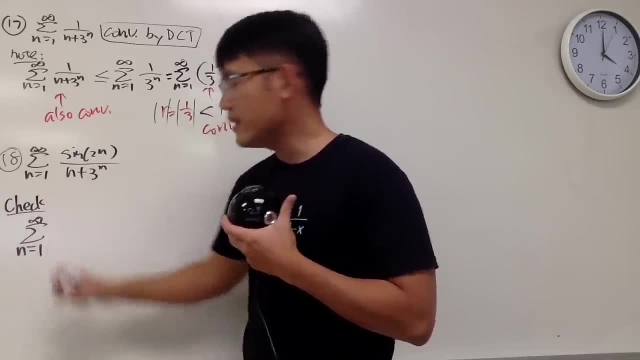 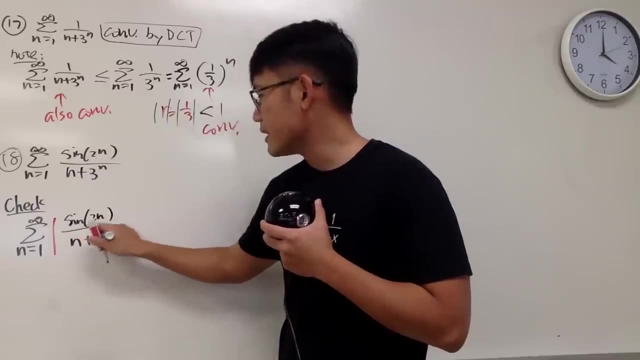 following The sum, as n goes from 1 to infinity, we will look at the absolute value of sine of 2n over n plus 3 to the nth power, Even though sometimes this the sine of 2n, sine of 2,. 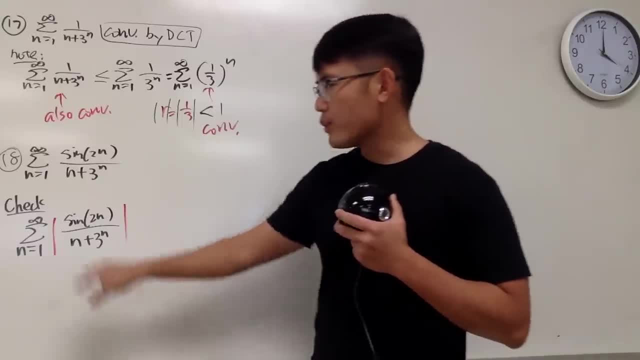 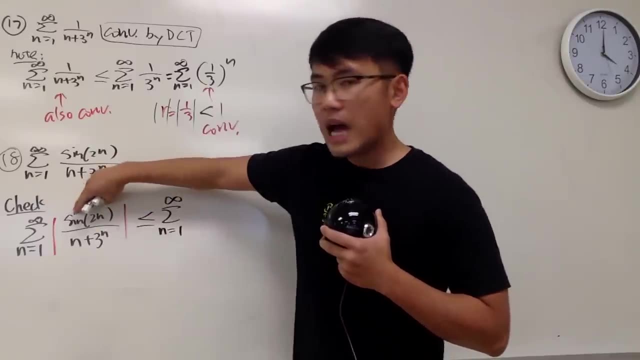 4,, 5, so on. that might be negative Absolute value. take care of that business. and we can say: this is destined equal to the sum, as n goes from 1 to infinity. Now the top is less than 1, so the whole fraction. 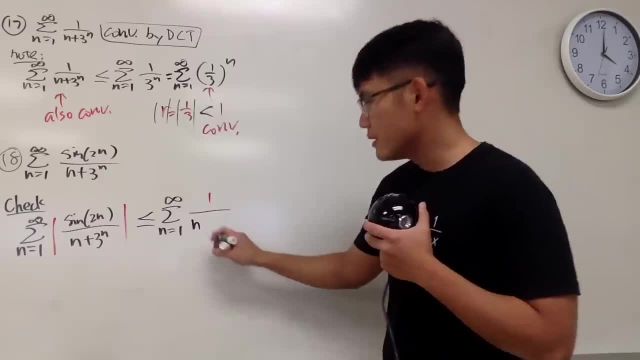 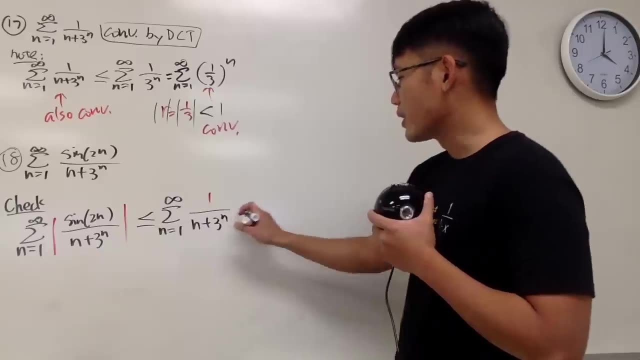 like: this is still, this is still less than that. So we have that And this becomes the question that we did earlier. but real quick, we can just say this right here: is less than or equal to the sum as n goes from 1 to infinity, 1 over. 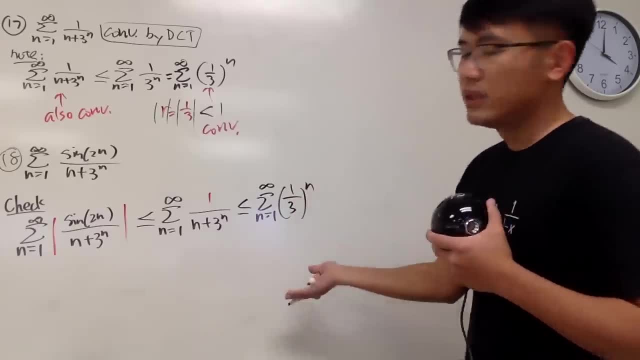 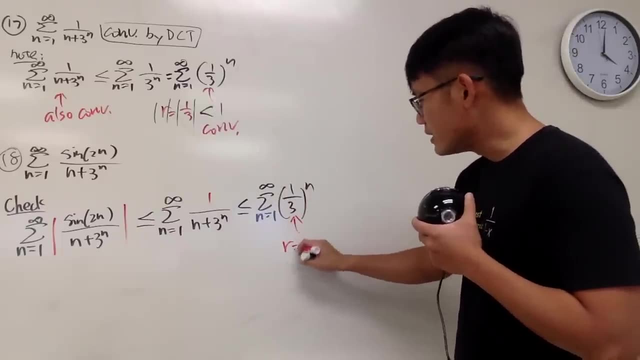 3 to the nth power. Especially if you have to do this question itself right, You cannot just say look back to question number 17.. Anyway, this right here you write down: r is equal to 1 third of the absolute value, which is less than 1,. 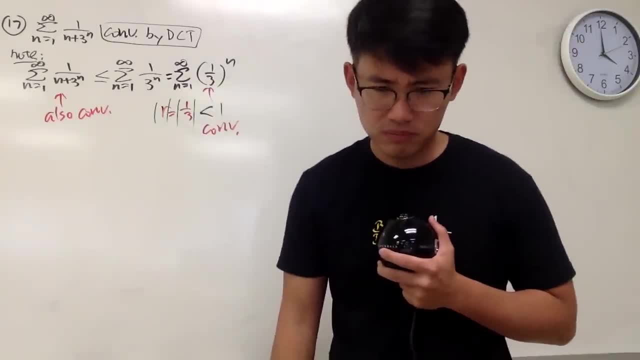 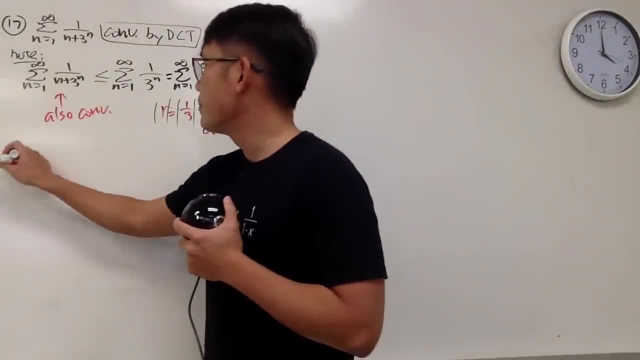 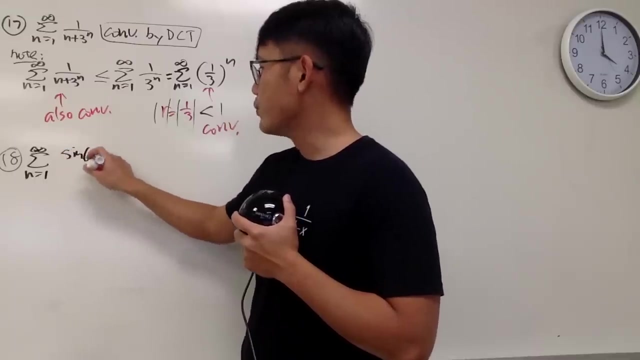 This is like that, easy Number 18.. Very similar Gosh. let's see Number 18.. We are going to do the sum as n goes from 1 to infinity, sine of 2n over and the bottom. here we have n. 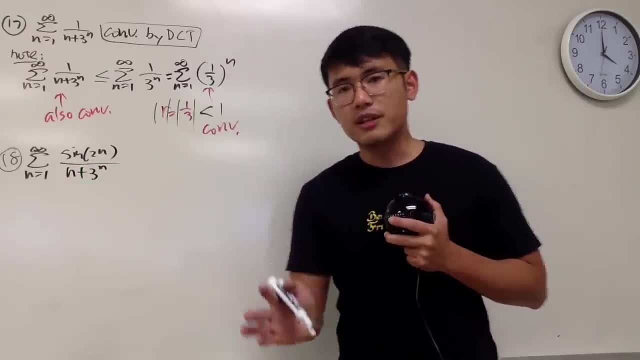 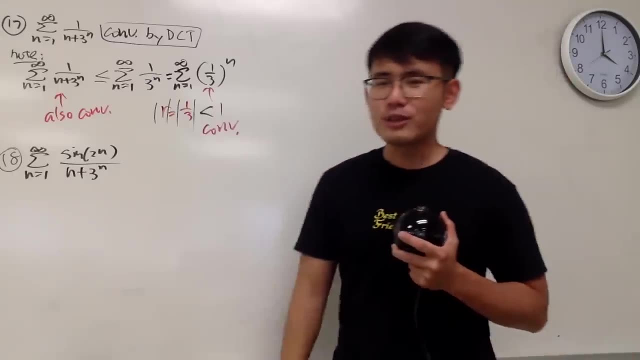 plus 3 to the nth power, like that. Remember what I told you guys earlier. When we see sine cosine in this kind of situations, what do we do? Just take the absolute value, Sometimes sine cosines, they cannot make up their minds. 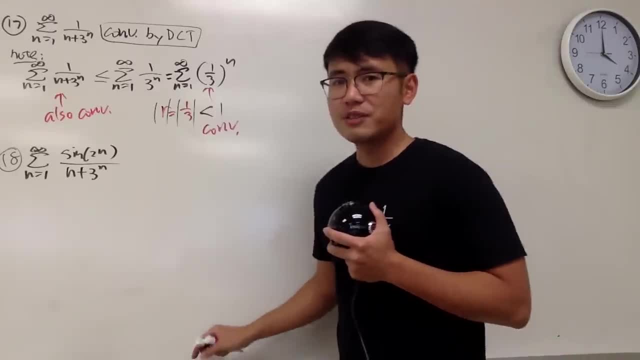 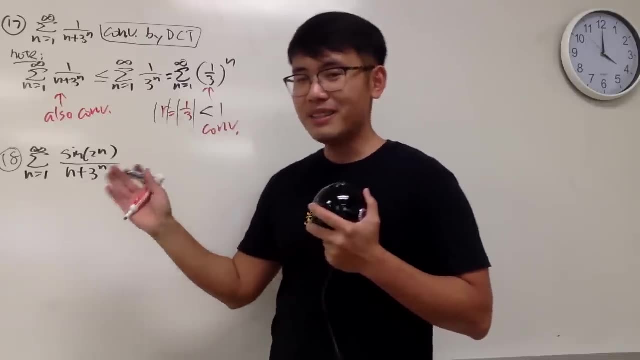 They will be negative sometimes. Don't let the negatives bother you. I will keep that in mind myself as well, because I do have haters. You guys don't know that, So I will keep that in mind. if necessary, I will put myself in absolute value. 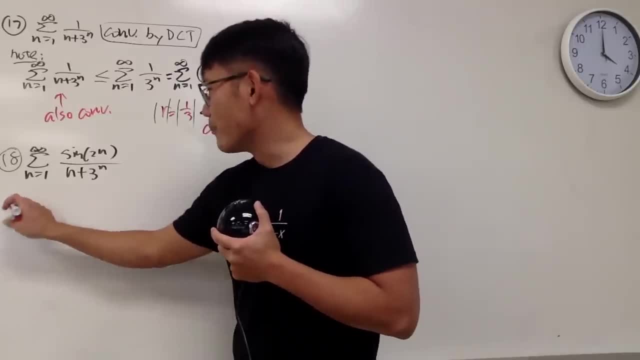 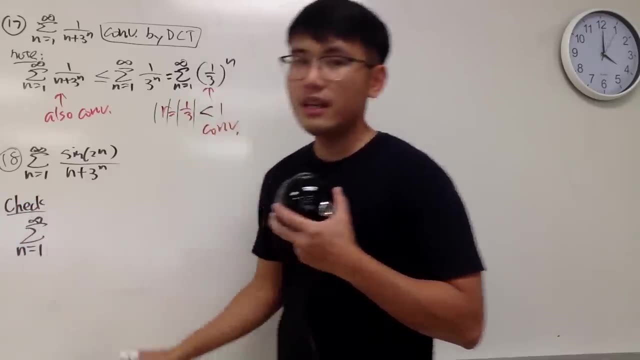 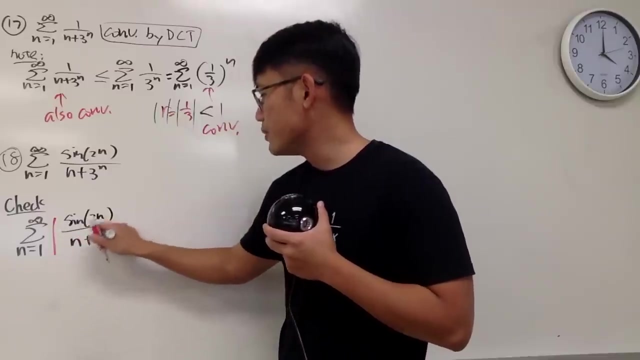 as a way to protect myself. Anyway, here we go. We are going to check the following: the sum as n goes from 1 to infinity. We will look at the absolute value of sine of 2n over n plus 3 to the nth power. 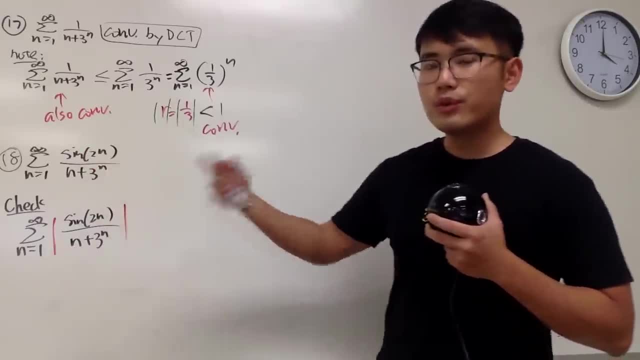 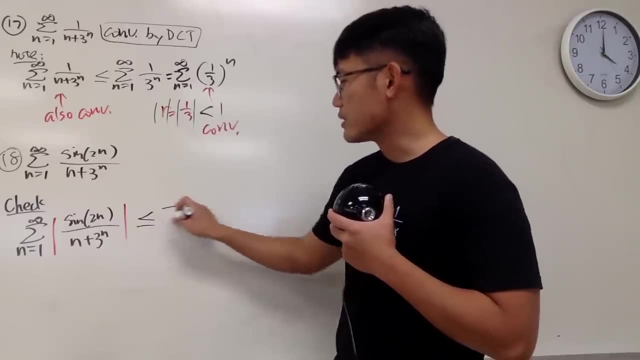 Even though sometimes this the sine of 2n, sine of 2,, 4,, 5 and so on, that might be negative Absolute value. take care of that business. and we can say this is less than or equal to the sum as n goes from 1 to infinity. 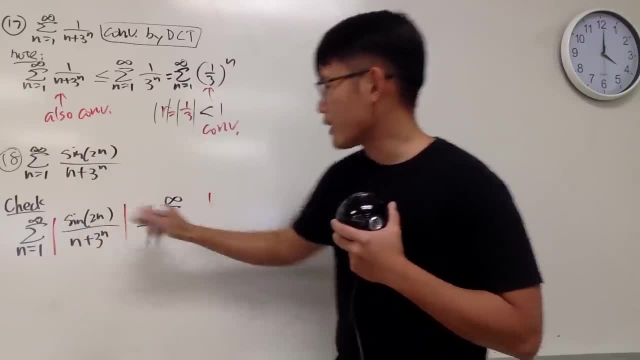 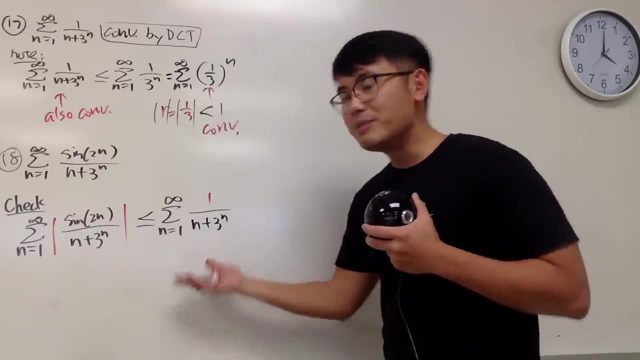 Now the top is less than 1.. So the whole fraction like this is still: this is still less than that. So we have that And this becomes the question that we did earlier. But real quick, we can just say this right here: is less than or equal to: 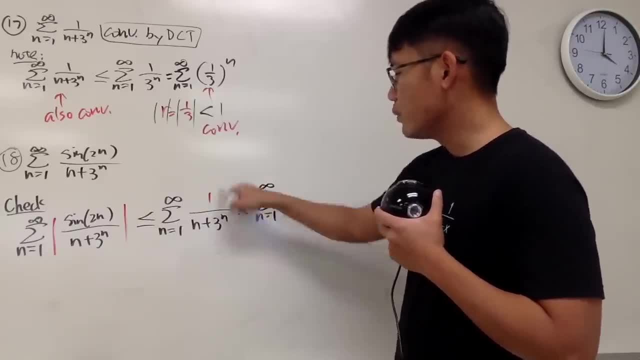 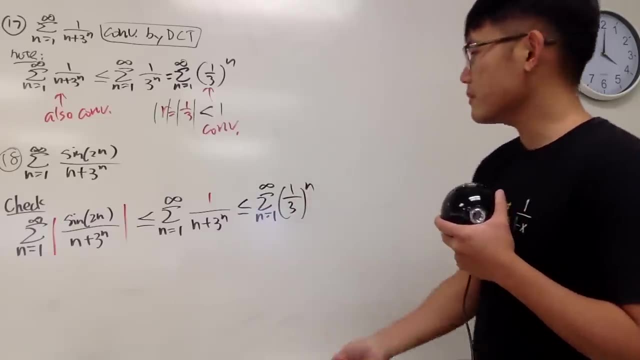 the sum as n goes from 1 to infinity, 1 over 3 to the nth power. Especially if you have to do this question itself right, You cannot just say look back to question number 17.. Anyway, this right here you write down: r is equal to 1 third. 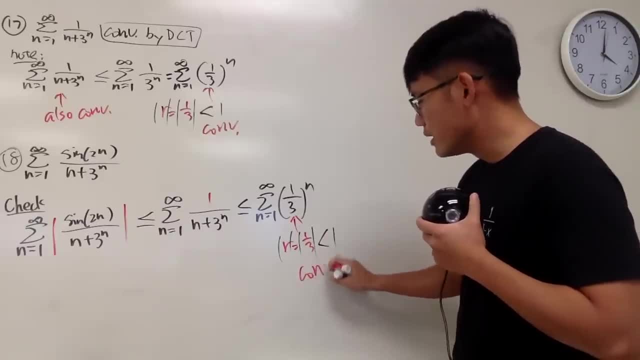 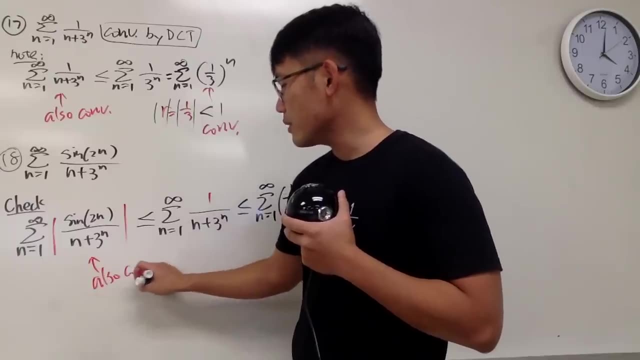 Take the absolute value, which is less than 1, which is a convergent, And now you can come back here and you can say this right here: also converges. And now here's the deal: You took the absolute value and it converges. 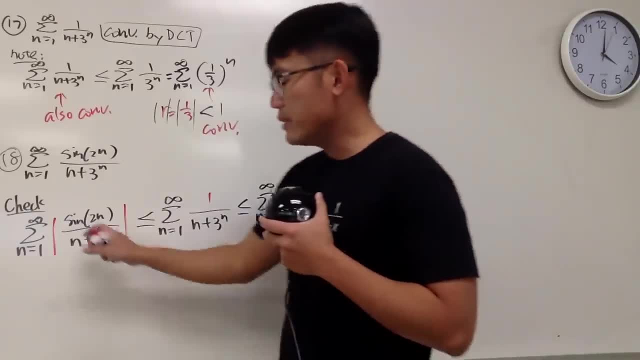 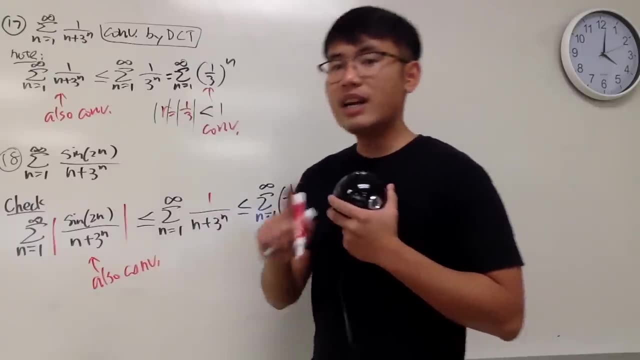 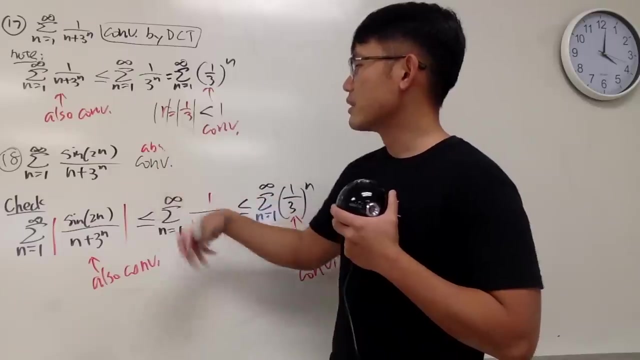 which is a convergent, And now you can come back here and you can say this right here: also converges. And now here's the deal. You took the absolute value and converges. You can say this right here: absolute converges. Up to you, though, depends on the question. 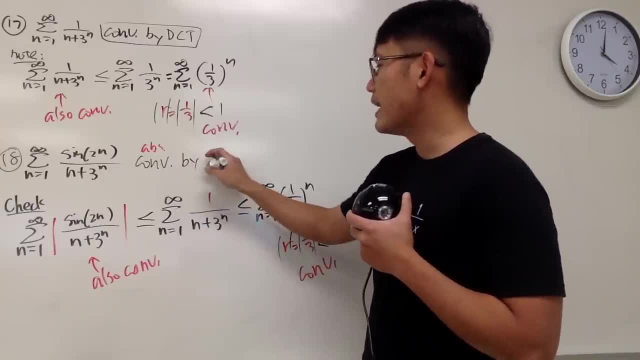 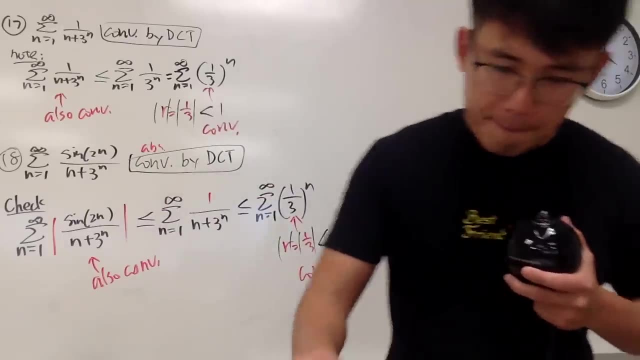 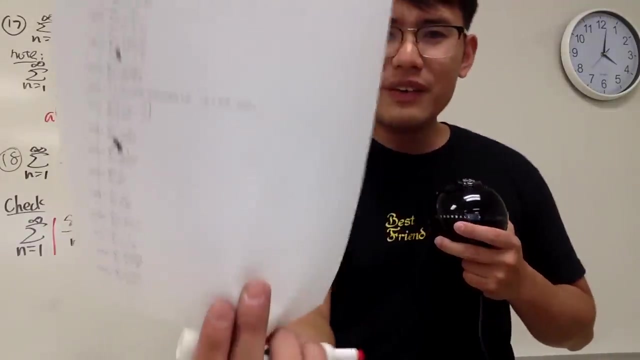 But you can just say this right here: converges, and again by the direct comparison test, And then we are done Just like that. Cool Now. Okay, very similar, number 19,. but that would be the first page. Oh, my god man. 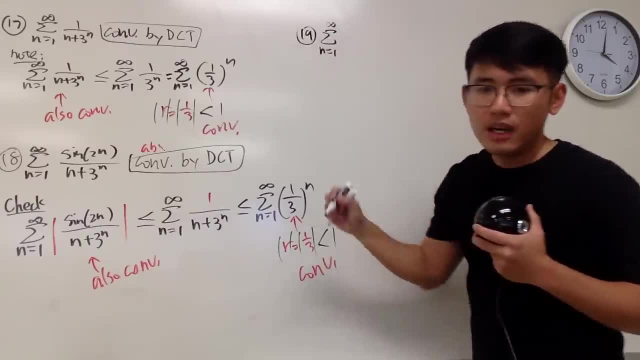 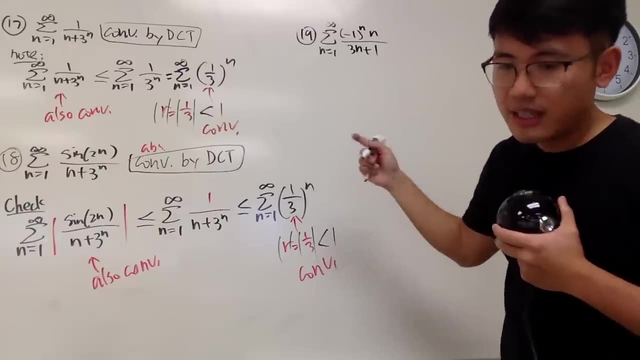 The sum as n goes from 1 to infinity and we have negative 1 to the nth power times, n over 3n plus 1, like this: Okay, we see negative 1, so this guy cannot make up his mind. Maybe sometimes it's positive. 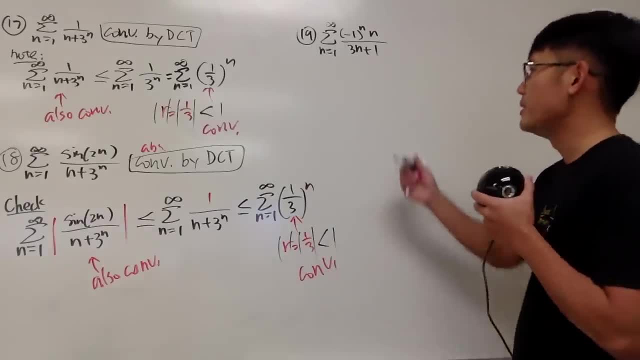 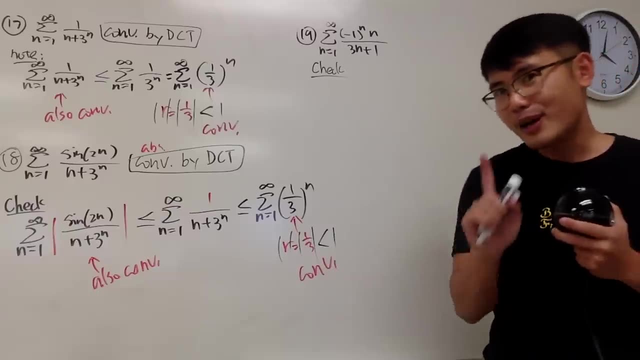 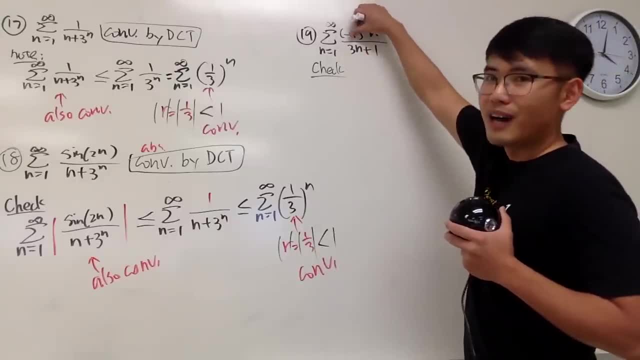 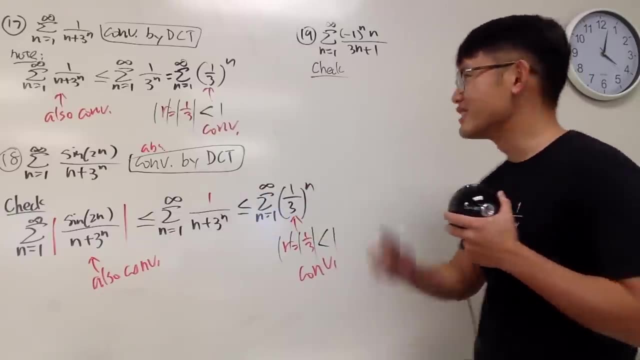 the absolute value. Even though I check the absolute value, this is gone, But you have n over 3n plus 1.. Does that approach 0? It doesn't. So we check the limit. We check the test for divergence. okay, Check. 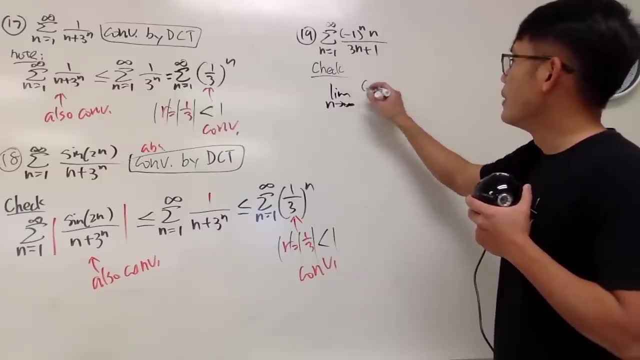 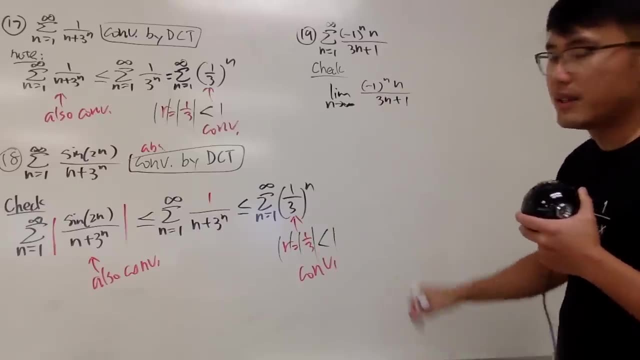 the limit, as n goes to infinity. And here we go: Negative 1 to the n, and this is n, 3n plus 1.. And here's the deal: When you take the limit right here, you just have to take care of the dominating power, which is the 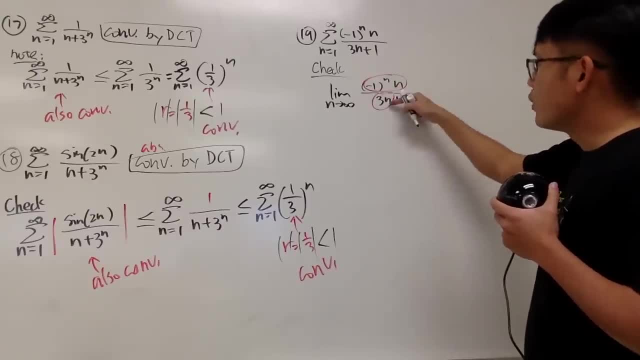 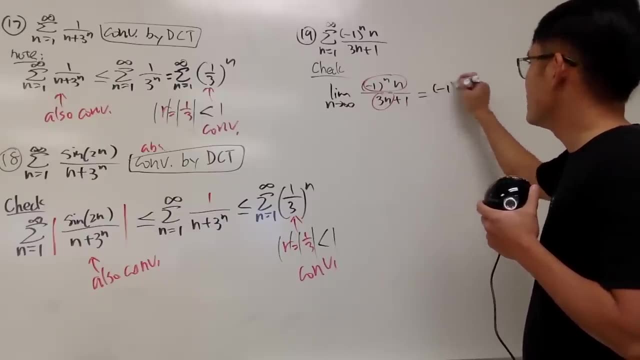 top over the bottom, the 1 doesn't really matter, And of course n over n is just, you know, 1 over 3, but it's like this: You can write it down like negative 1, and then you have the infinity. 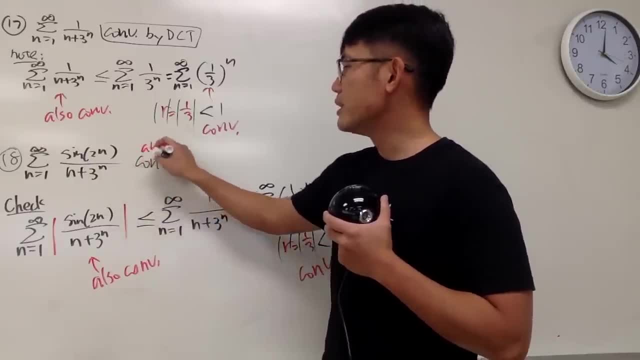 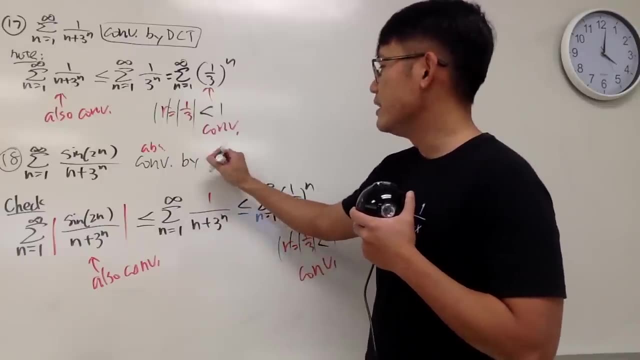 You can say this right here: Absolute converges. Up to you though, Depends on the question, But you can just say this right here: Converges, And again by the direct comparison test, And then we are done Just like that. 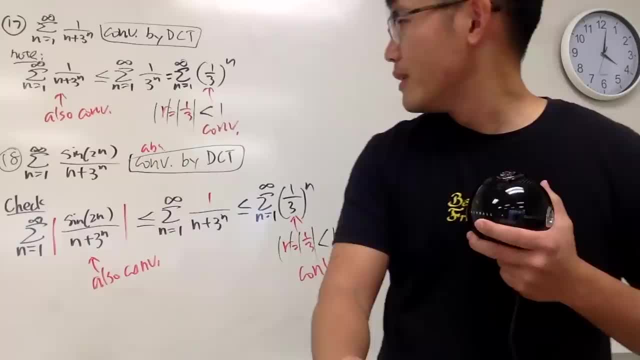 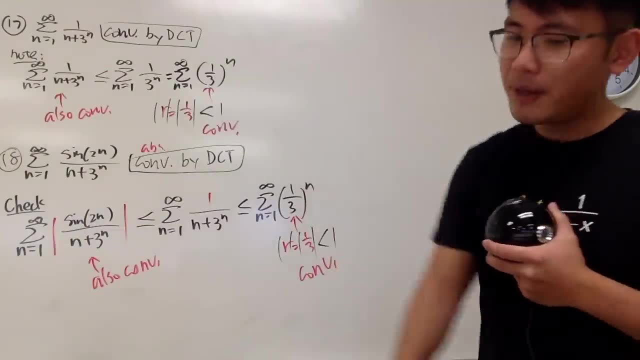 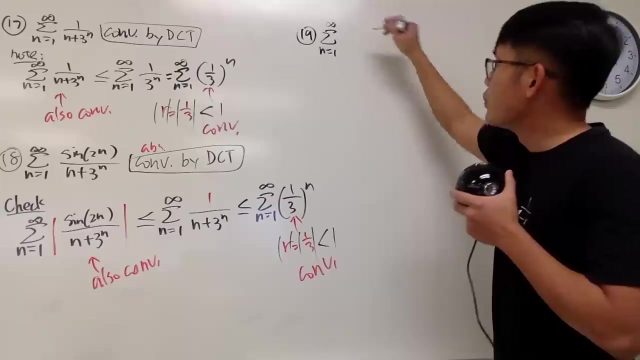 Cool. Now let's look at question number 19.. Okay, Very similar number 19.. But that will be the first page. Oh, my god man, The sum as n goes from 1 to infinity And we have negative 1 to the nth power. 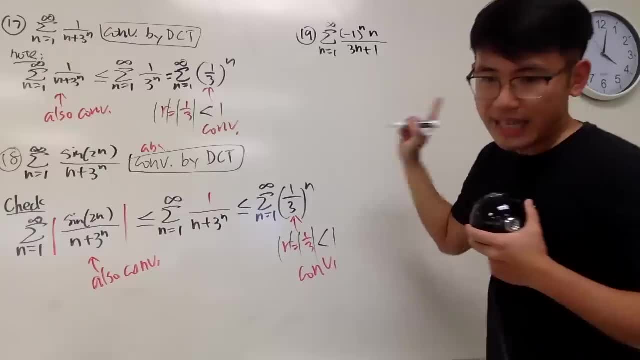 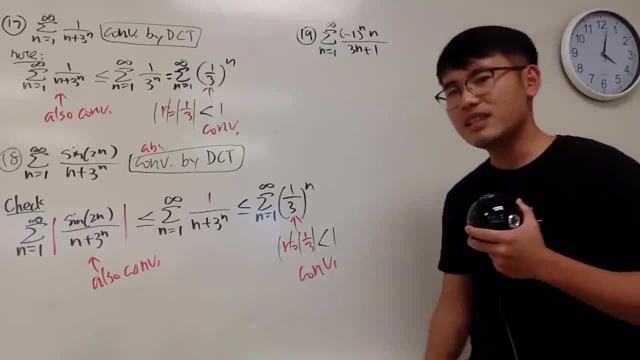 times n over 3n plus 1.. Like this, Okay, We see negative 1.. So this guy cannot make up his mind. Maybe sometimes it's positive, Maybe sometimes it's negative, Don't worry, Take the absolute value. 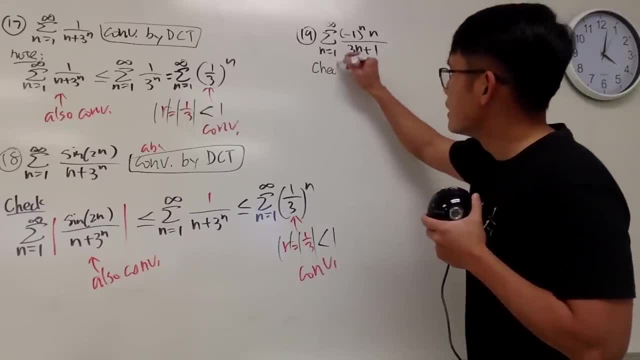 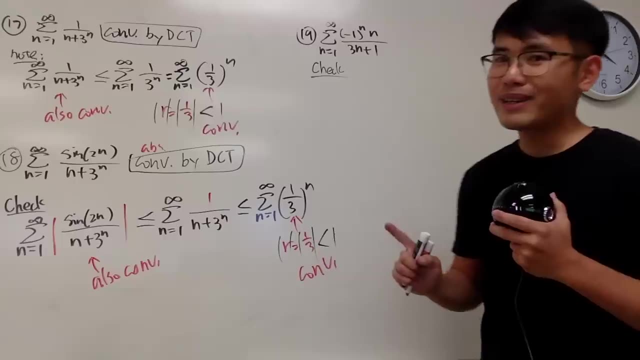 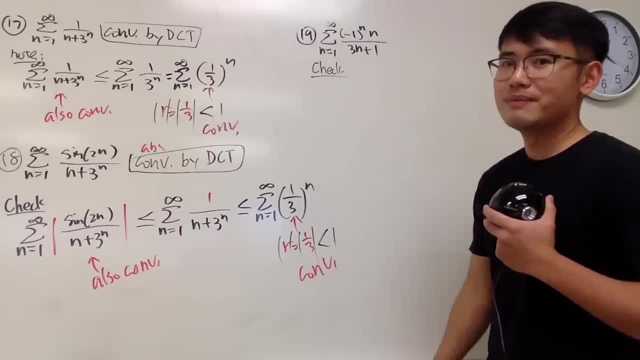 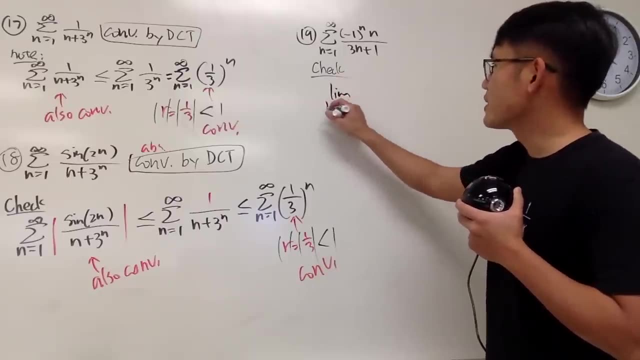 But we have n over 3n plus 1.. Does not approach 0. It doesn't. So we check the limit. We check the test for divergence. Okay, Check the limit as n goes to infinity. And here we go. 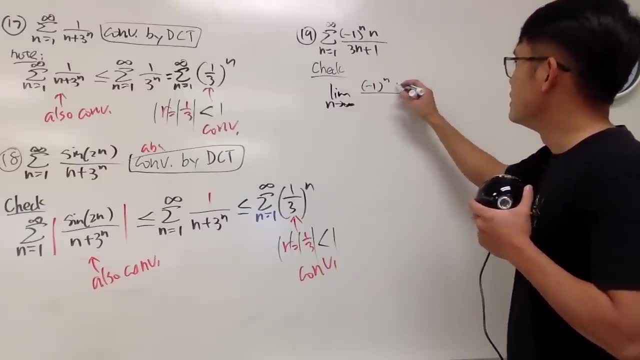 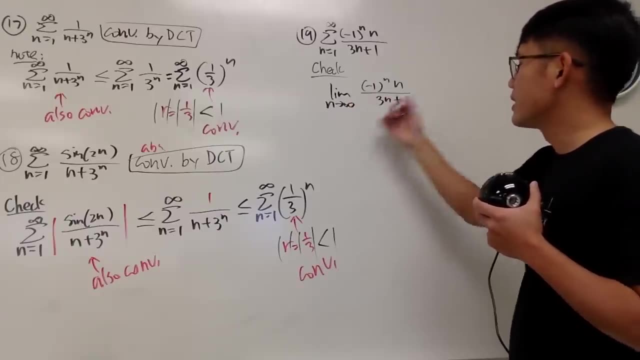 Negative 1 to the nth power to the n, and this is n, 3, n plus 1.. And here's the deal. When you take the limit right here, you just have to take care of the dominating point, which is the top over the bottom. 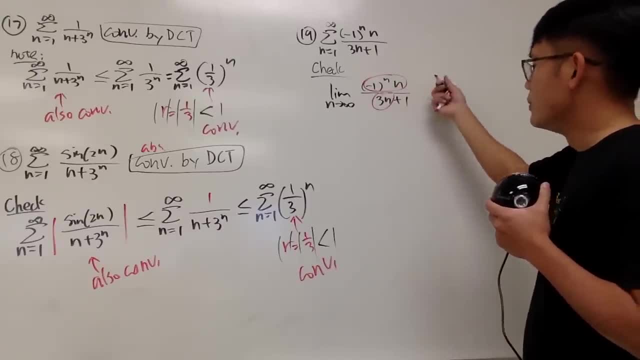 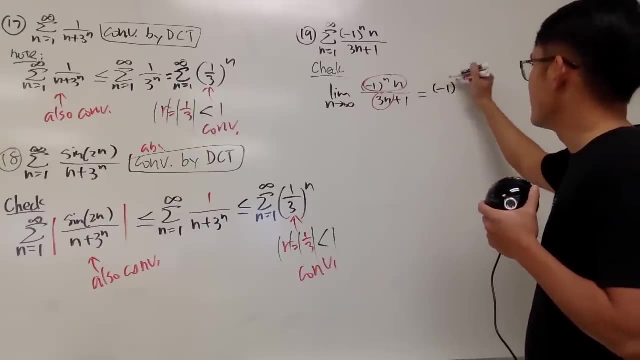 the 1 doesn't really matter, And of course n over n is just, you know, 1 over 3, but it's like this: You can write it down like negative 1, and then you have the infinity, and then you have this. 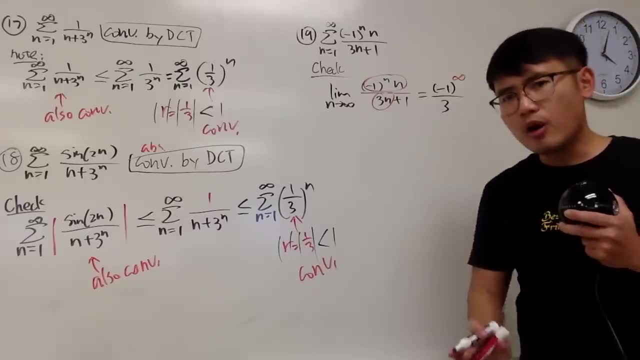 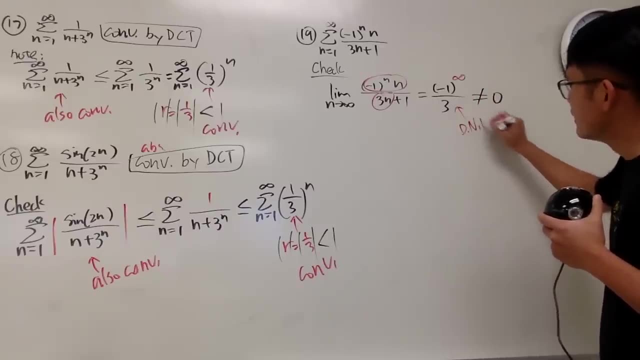 and then you have this right here, it's just 3.. But all in all, this guy right here is not equal to 0. Technically, this right here, the limit does not exist. Alright, This right here does not exist. 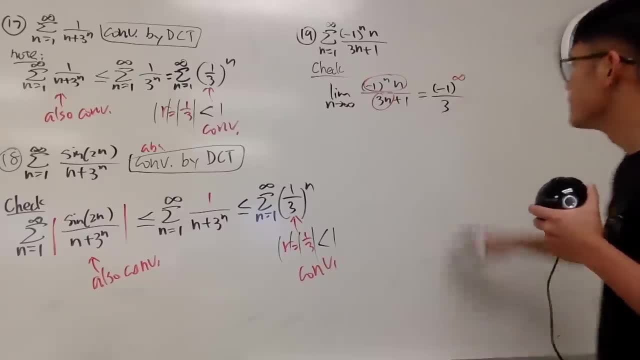 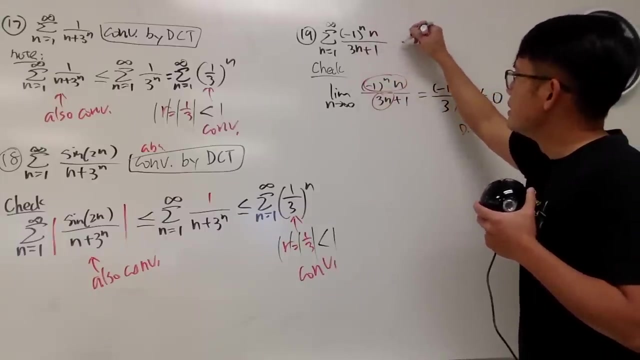 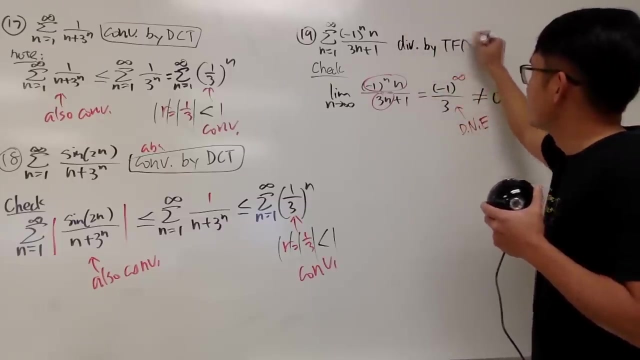 right here is just 3.. But all in all, this guy right here is not equal to 0. Technically, this right here the limit does not exist. right, This right here does not exist. So you can come back here and say this series diverges, this right here diverges, by the test for divergence, like that. 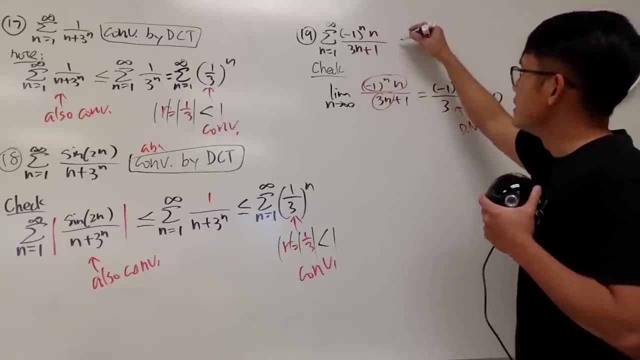 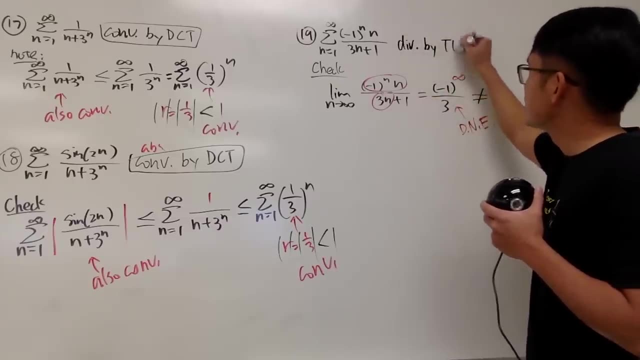 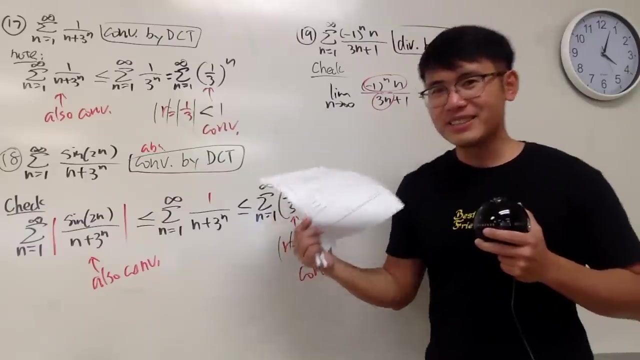 So you can come back here and say this series diverges, This right here diverges by the test for divergence, Like that. And then we've got that. God, Oh my god, this took me so long to do the first page And 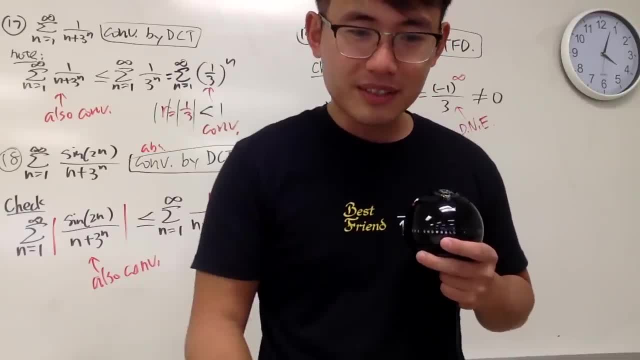 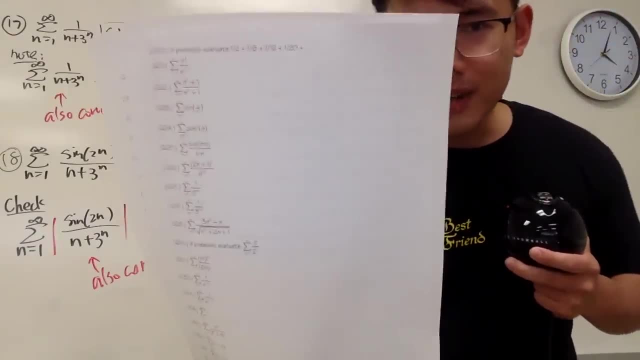 because I did another part earlier and I wasn't satisfied with that, so I'm doing this again. Yeah, that's just life. Okay, number 20.. Congratulations. we're going to compute some actual limits, So we will see. this is number 20. 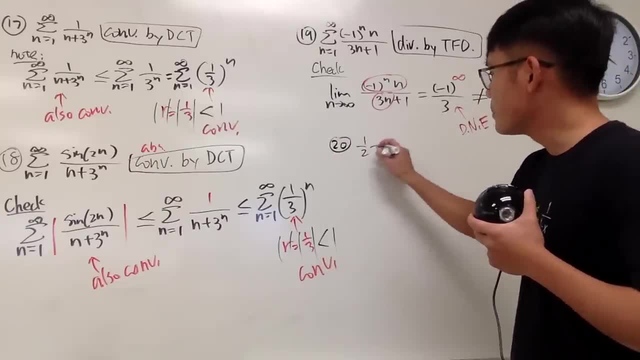 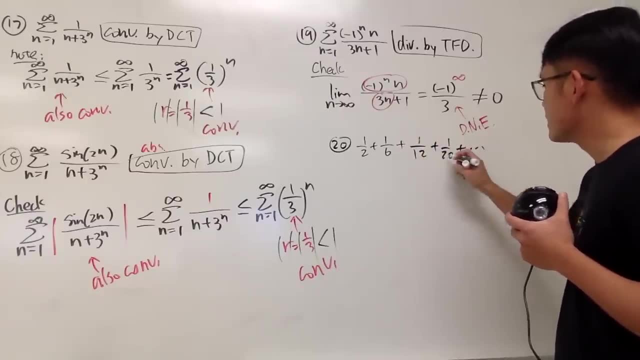 here and we will have to calculate 1 half plus 1 over 6, plus 1 over 12, plus 1 over 20, plus dot dot dot and all that. Hmm, You can pause the video and think about it. This is a rather challenging question. 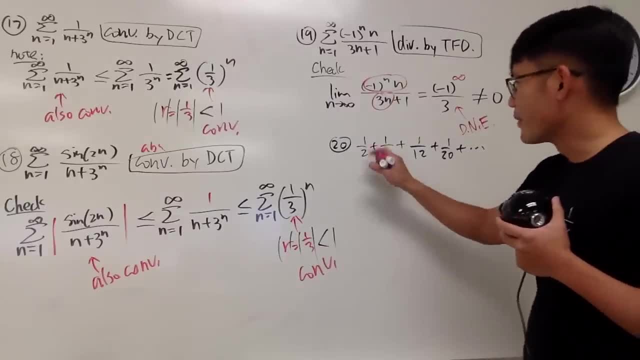 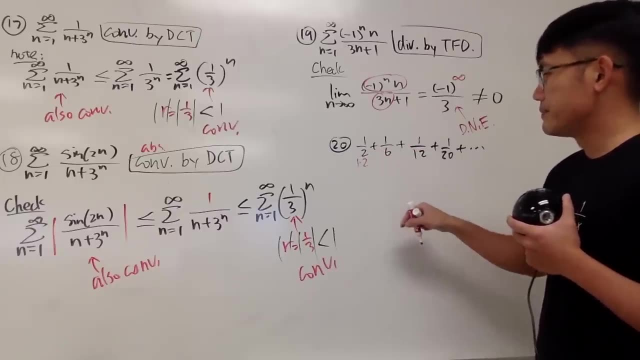 Okay, Okay, here we go n start with 1, you can just take that and you see, this 2 is the same as saying 1 times 2.. This 6 is like saying 2 times 3.. This 12 is the same as. 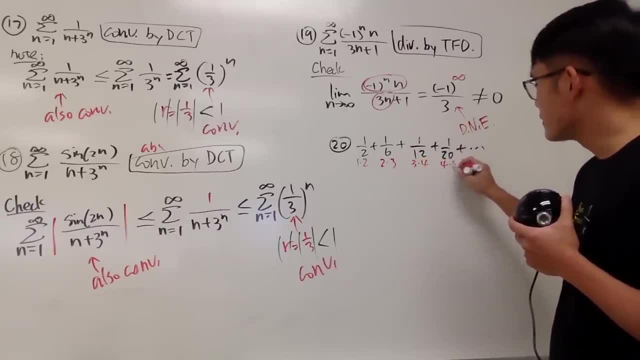 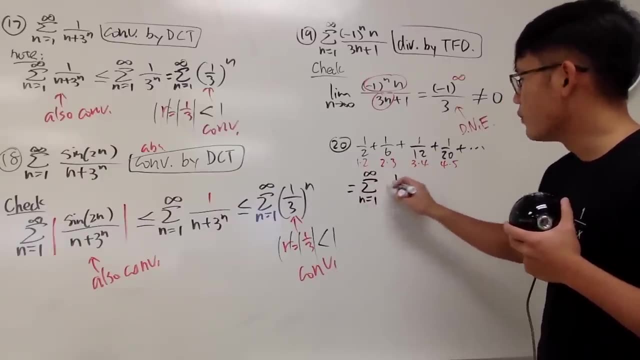 saying 3 times 4.. And this right here is like saying 4 times 5, and so on. So you can actually write this down as the sum as n goes from 1 to infinity, of 1 over n times n plus 1.. 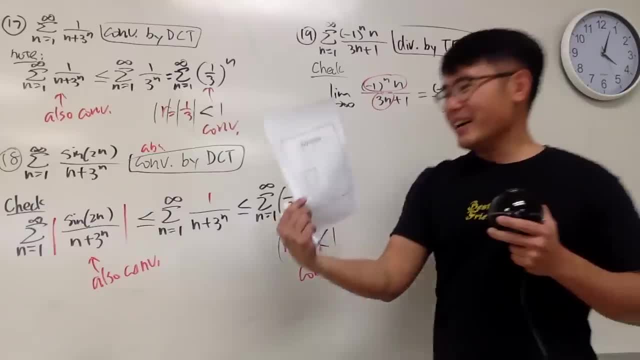 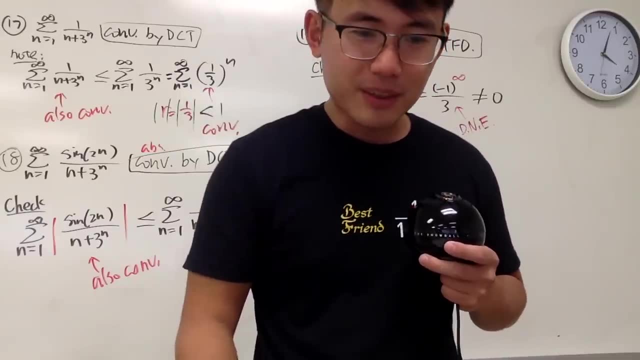 Look at that, God. Oh my god. this took me so long to do the first page And because I did another part earlier and I wasn't satisfied with that, so I'm doing this again. Yeah, that's just life. 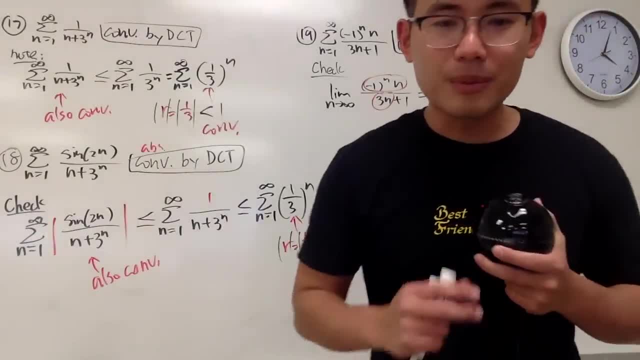 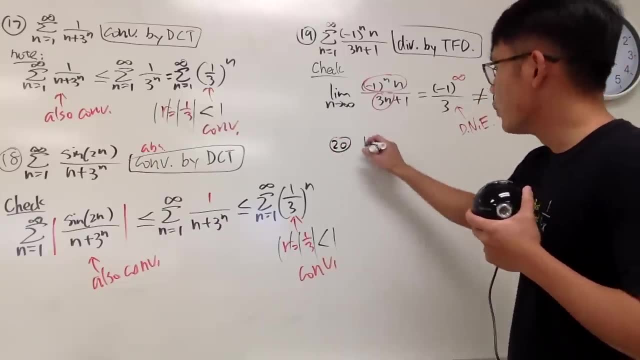 Okay, number 20.. Congratulations, we're going to compute some actual limits, So we will see. this is number 20 here and we will have to calculate 1 half plus 1 over 6 plus 1 over 12 plus 1 over. 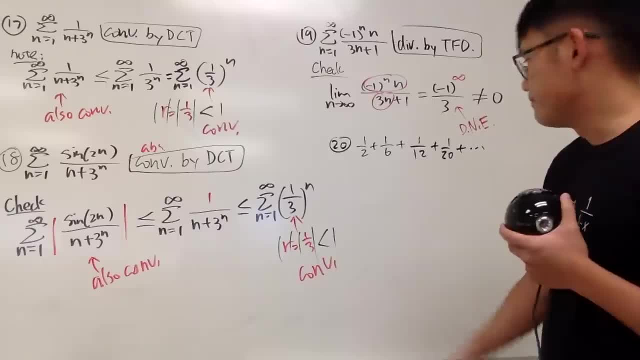 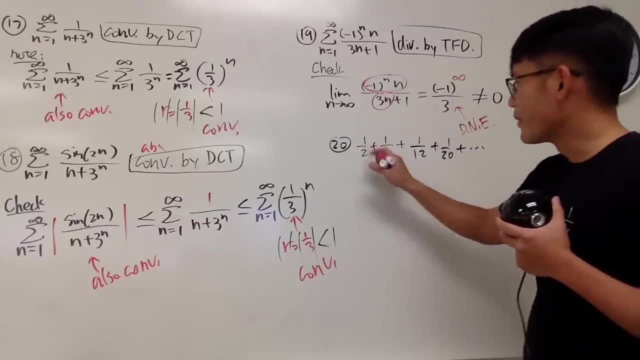 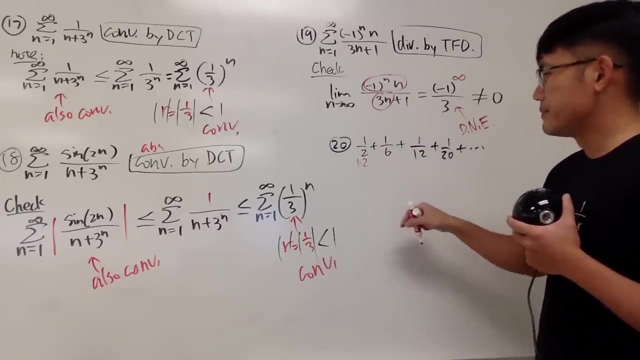 20 plus dot, dot, dot and all that. Hmm, you can pause the video and think about it. This is a random, challenging question, Okay, Okay, here we go. Unstart with one. You can just take that and you see this 2 is the same as saying 1 times 2.. This 6 is saying 2 times 3.. 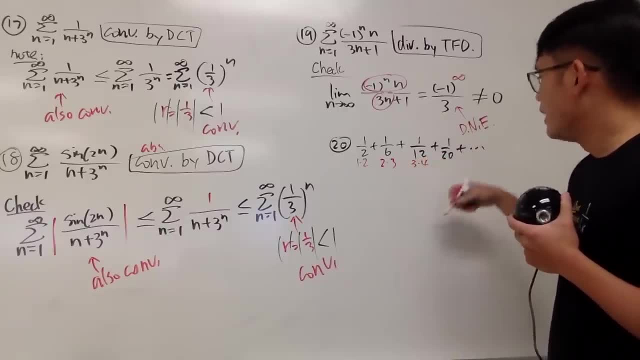 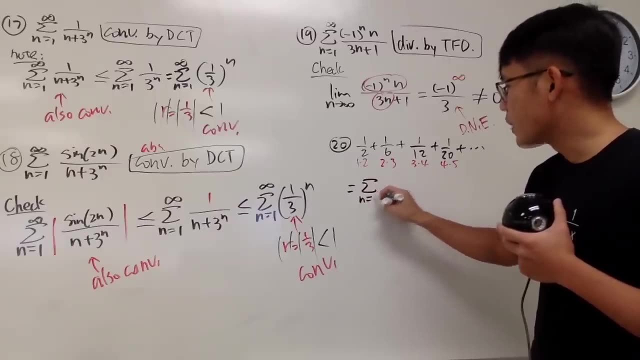 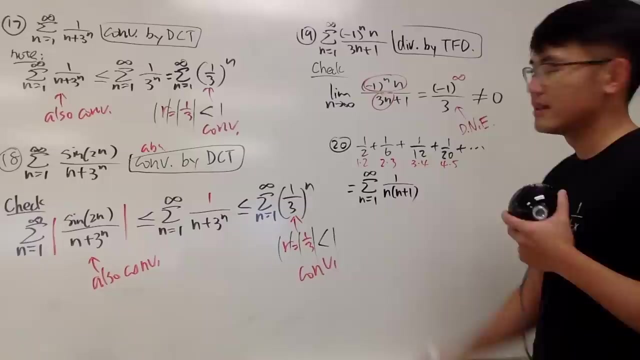 This 12 is the same as saying 3 times 4,, and this right here is saying 4 times 5, and so on. So you can actually write this down as the sum- sum, as n goes from 1 to infinity, of 1 over n times n plus 1, isn't it? And this right? 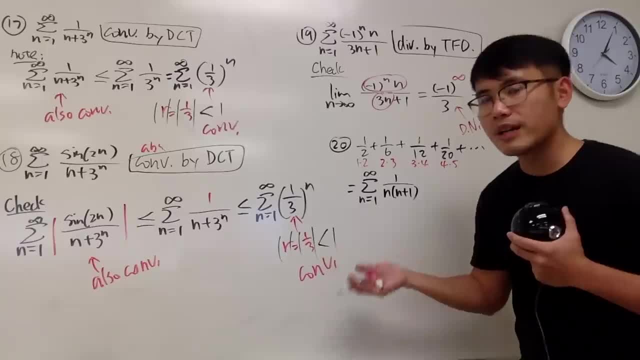 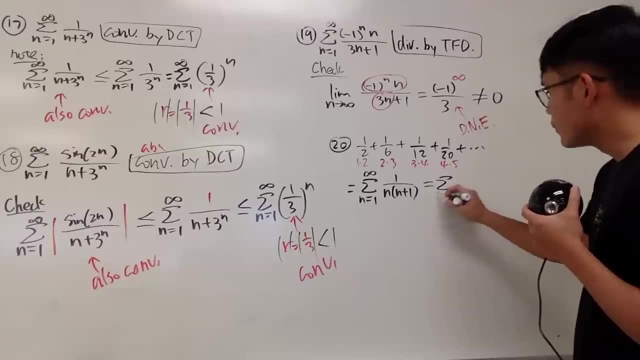 here it does converge, but we actually calculate the actual value right here, and to do so we will have to use partial fractions. And let me show you real quick. we take the sum: as n goes from 1 to infinity, the first guy has something over n, and then the next guy. 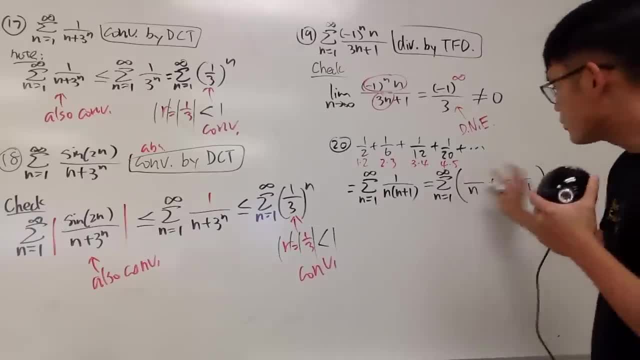 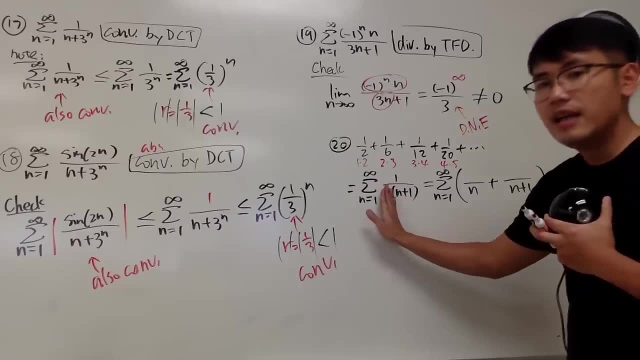 has something over n plus 1.. This time, this right here is going to be of the same kind. you will see Here we go To figure this out. I will come back here and cover this and I will have to let n equal to 0, put that 0 into here. 1 over 0 plus 1 is just 1, so 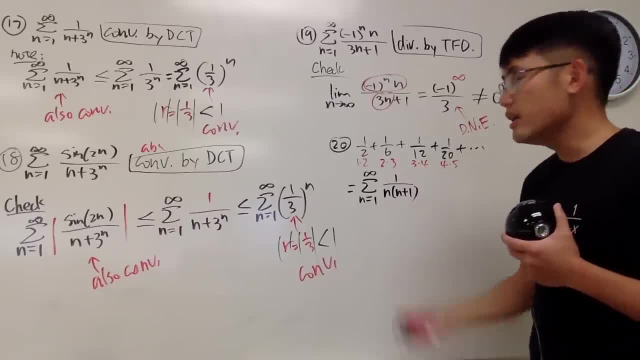 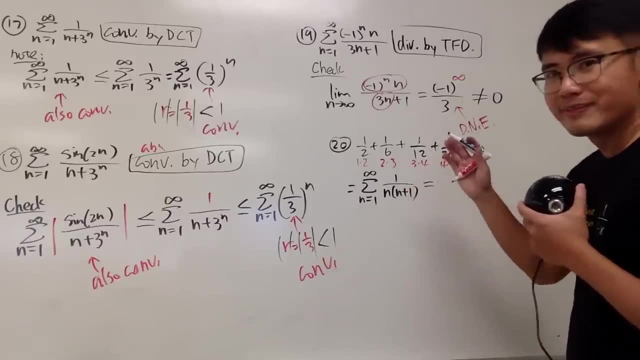 Isn't it? And this right here it does converge, but we actually calculate the actual value right here, And to do so we will have to use partial fractions. And let me show you real quick. We take the sum as n goes from 1 to infinity. 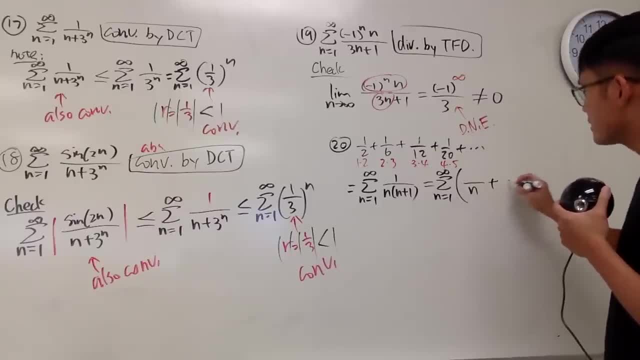 The first guy has something over n, and then the next guy has something over n plus 1.. This time, this right here is going to be of the same kind. you will see, Here we go To figure this out. I will come back here and cover this. 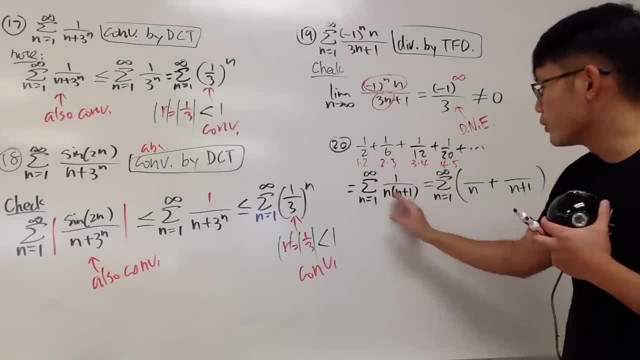 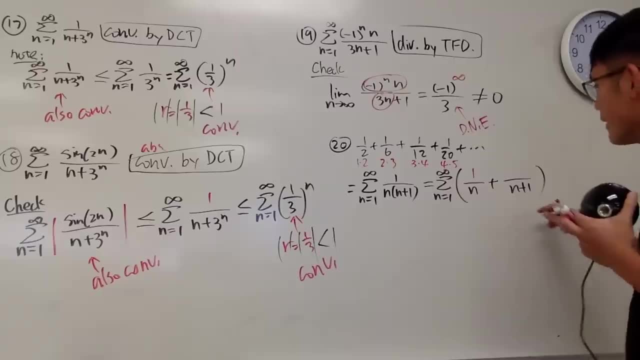 And I will have to let n equal to 0. Put that 0 into here: 1 over 0 plus 1 is just 1.. So that's nice. Huh, So we have the 1 right here Now. 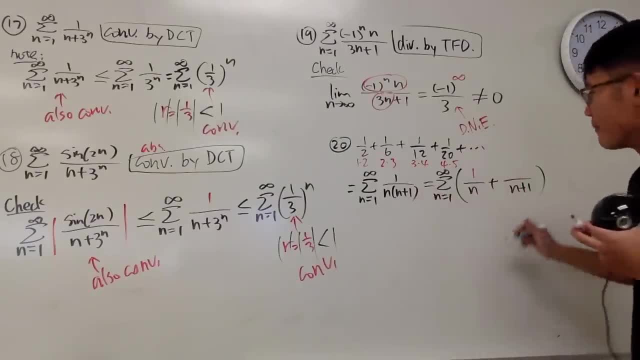 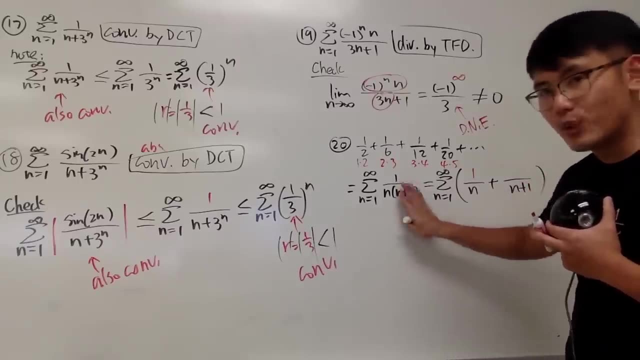 that's nice. So we have the 1 right here Now. well, I have to figure this out. come back here, cover this. I have to let n equal negative 1 to kill this term. Putting negative 1 here. 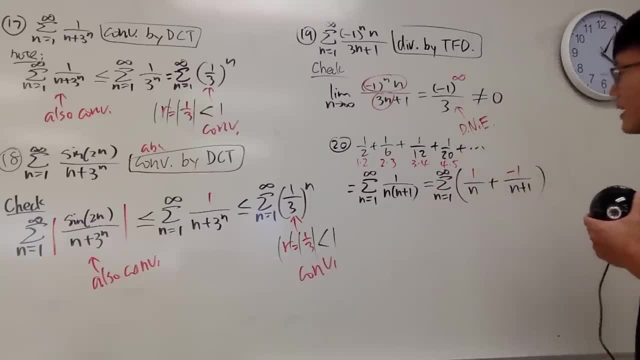 1 over negative 1, we get negative 1, so we have a minus 1, like this. So, as you can see, this is a telescoping series and I will just write down a few terms for you guys, you guys. 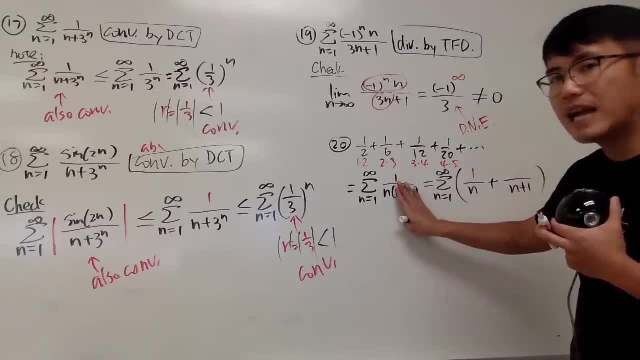 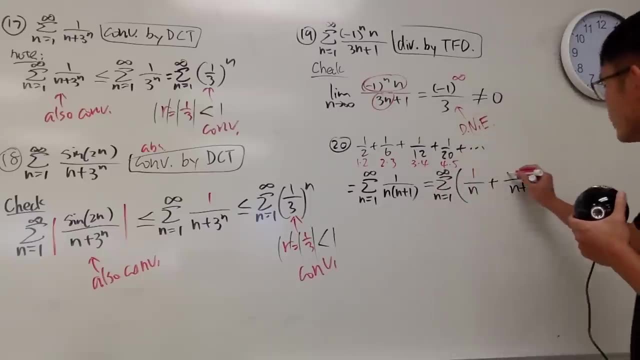 well, I have to figure this out. Come back here, cover this. I have to let n equal negative 1 to kill this term. Putting negative 1 here, 1 over negative 1, we get negative 1.. So we have a minus 1, like this: 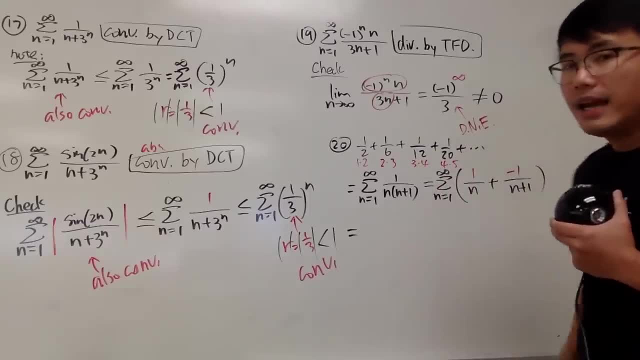 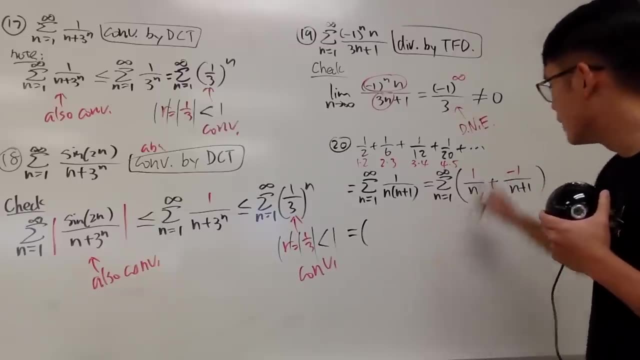 So, as you can see, this is a telescoping series And I will just write down a few terms for you guys. You guys will see what's up with this. The first term: with this parenthesis, we will get 1 over 1. 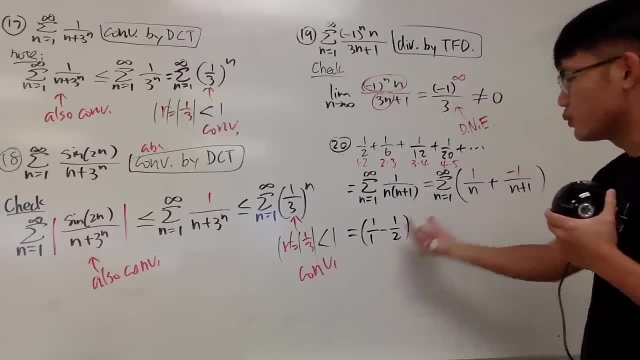 minus 1 over 2.. In this parenthesis, when n is equal to 1.. Next we add as n goes. as n is equal to 2, put the 2 here, we get 1 over 2 minus 1 over 3.. 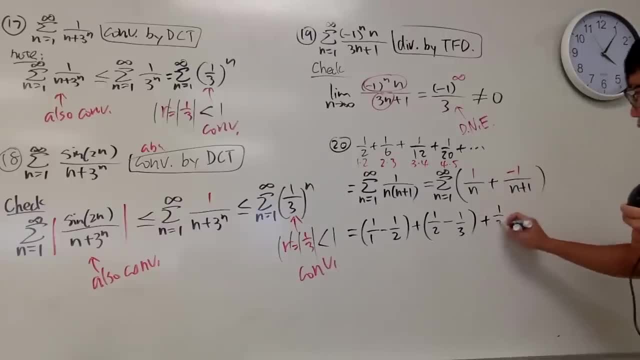 And then so on. Plus, the third one is going to be 1 over 3 minus 1 over 4.. And then so on, so on, so on, And technically you will have to put down the nth term right here. 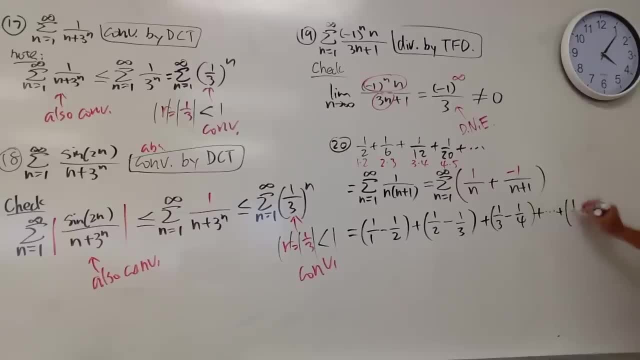 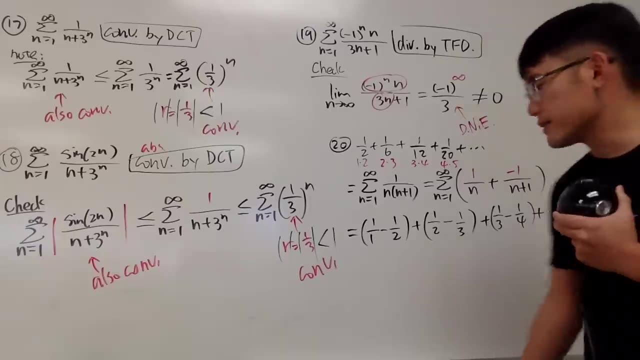 Plus 1 over n minus 1 over n plus 1.. Like this? Alright, And now check this out For the first parenthesis. you will see that, okay, this stays, but this right here will be cancelled with that. so this: 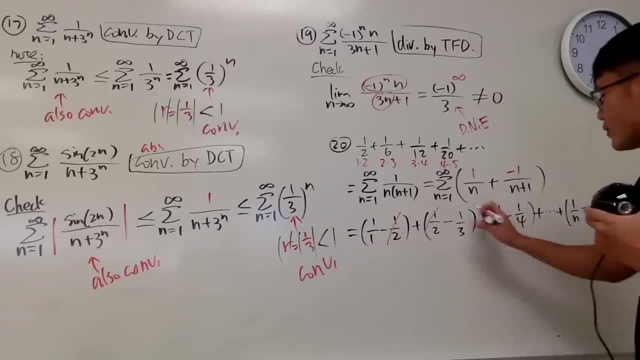 and that- cancel And check this out. This and that also cancel, and this right here also cancel, and so on. And at some point, you know, this will be cancelled, with some in the front, and this right here will be the nth term and it stays. 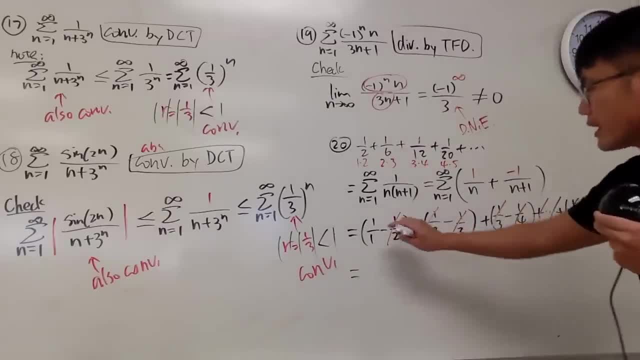 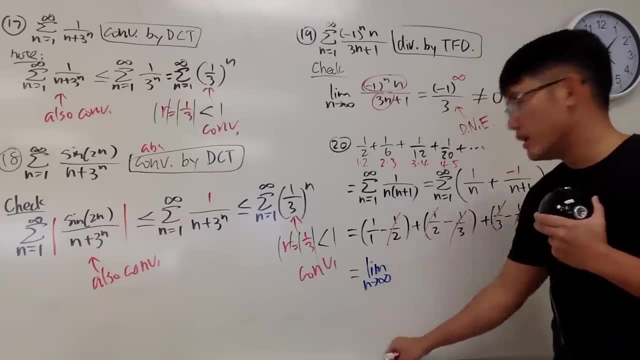 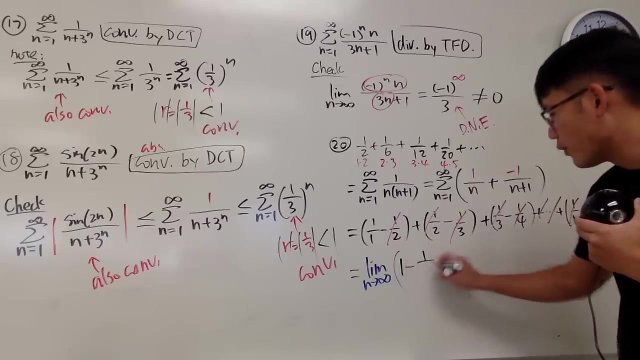 And we have to do the following. This right here is the nth partial sum. We will have to take the limit as n goes to infinity, and we'll see the remaining part, which is 1 minus 1 over n plus 1.. Like this. 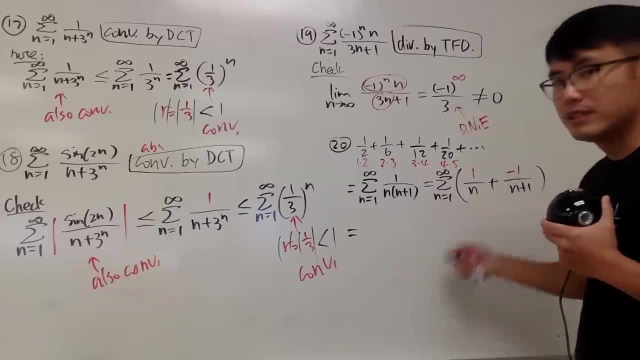 will see what's up with this. The first term: with this parenthesis we will get 1 over 1 minus 1 over 2.. In this parenthesis, when n is equal to 1.. Next we add as n is equal. 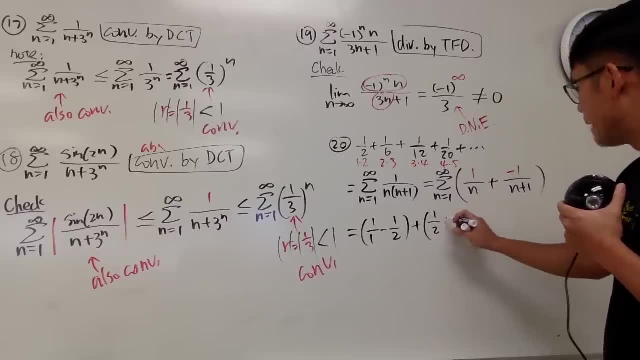 to 2, put the 2 here, we get 1 over 2 minus 1 over 3.. 1 over 3 minus 1 over 4.. And then so on, and then so on. Plus, the third one is going to. 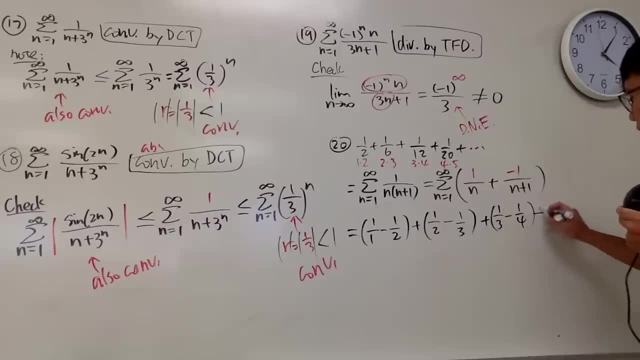 be 1 over 3, minus 1 over 4, and then so on, so on, so on, And technically you will have to put down the nth term right here: plus 1 over n minus 1 over n plus 1.. Like this: 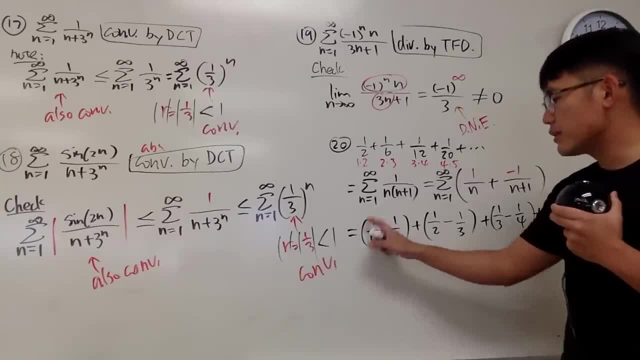 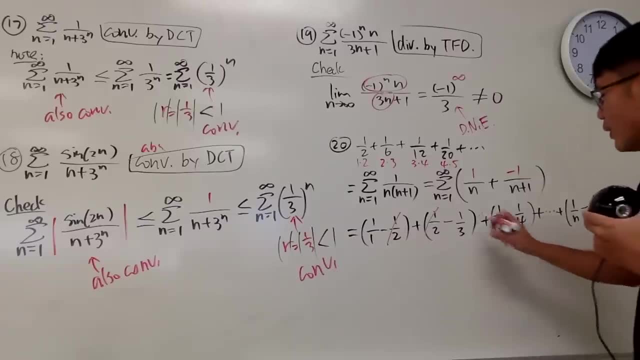 alright, And now check this out. For the first parenthesis, you will see that, ok, this stays, but this right here will be cancelled with that. so this and that cancel, and check this out. this and that also cancel, and this right here also cancel, and so on, and at some point you 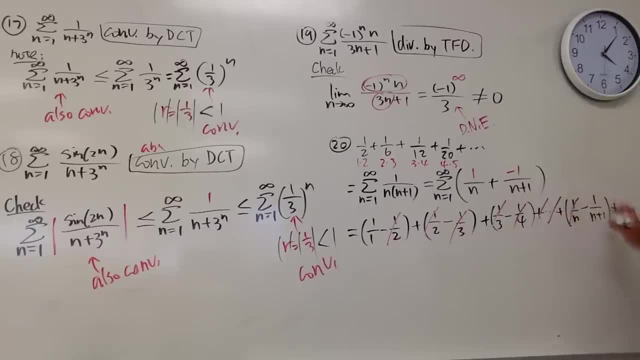 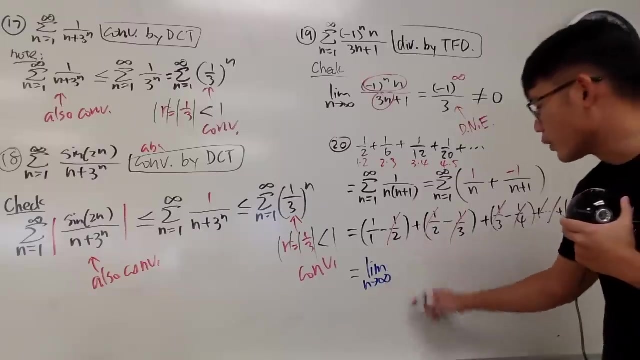 know this will be canceled with something in the front and this right here will be the nth term and it stays and we have to do the following: this right here is the nth partial sum. we will have to take the limit as n goes to infinity and we'll see the remaining part, which is 1 minus. 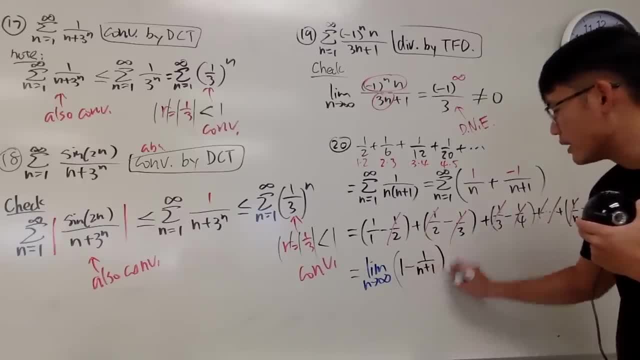 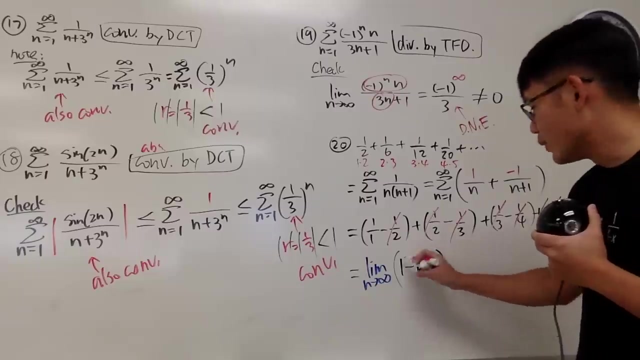 1 over m plus 1, like this, and you guys know i will change the color back. that was the wrong one. okay, all right, so we have this right here. right, and of course, once you put the infinity here, we do end up with 1 minus 1 over infinity. 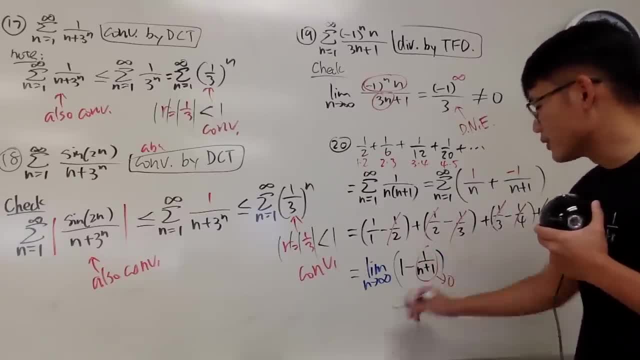 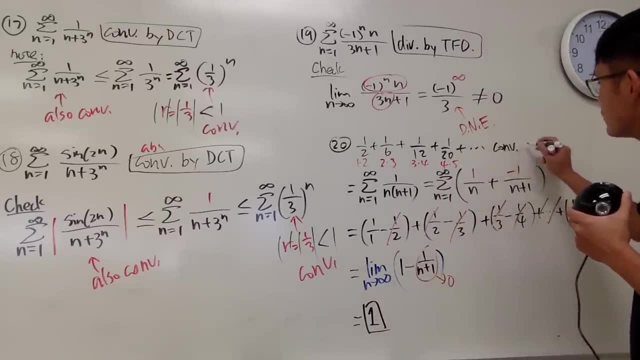 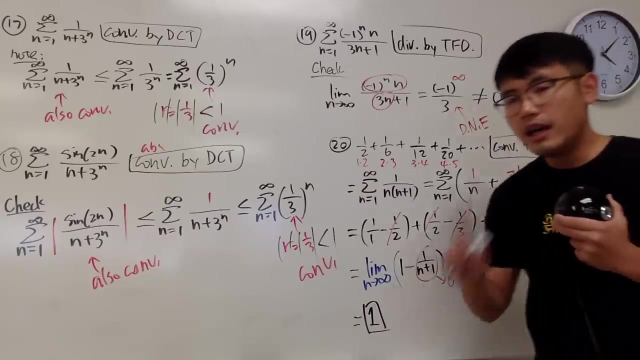 plus 1, which is just, you know, going to 0. so in another word, all in all we get the answer is 1. so we can say this right here: actually come converges to 1, right, so the answer is just 1, very cool telescoping series and another. 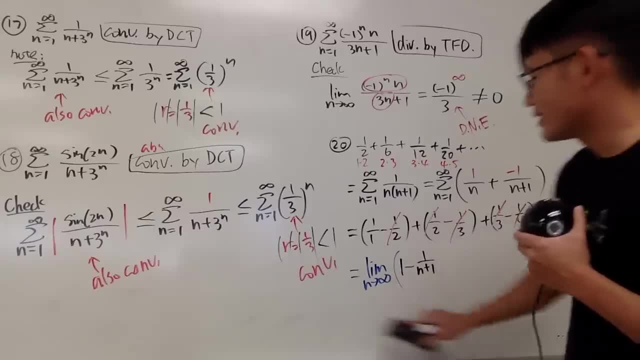 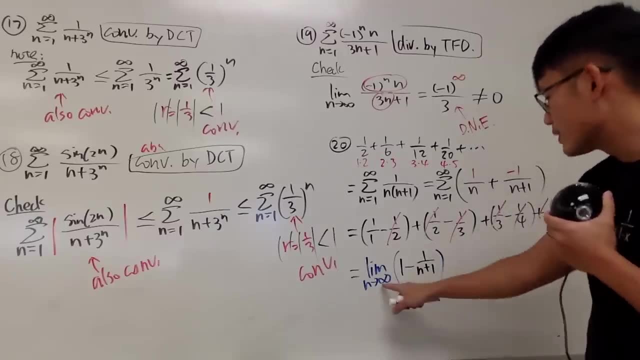 And you guys know I will change the color back. That was the wrong one. Alright, So we have this right here, Right? And of course, once you put the infinity here, we do end up with 1 minus 1 over infinity plus 1, which. 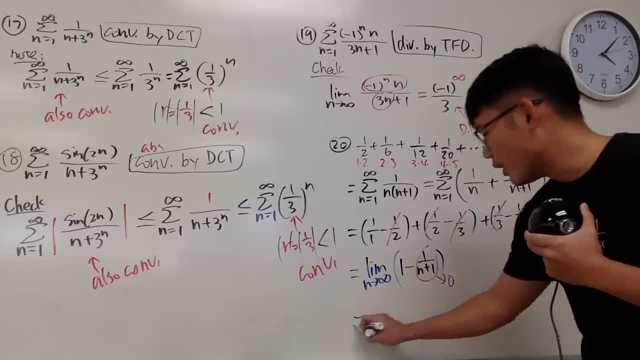 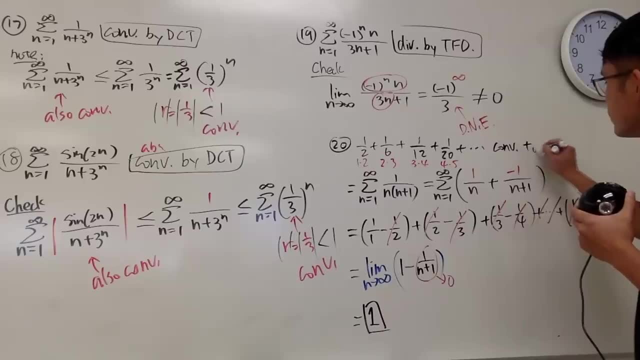 is just, you know, going to 0.. So in another word, all in all we get, the answer is 1.. So we can say this: right here actually converges to 1.. Right, So the answer is just 1.. 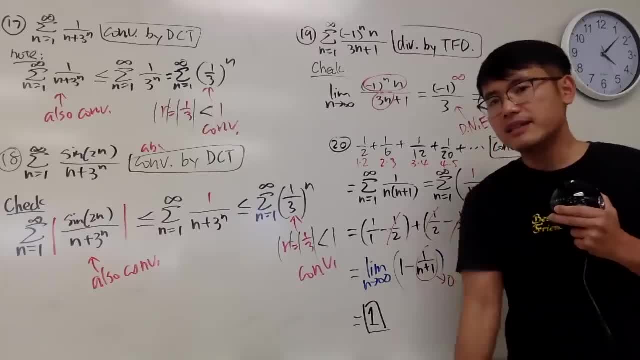 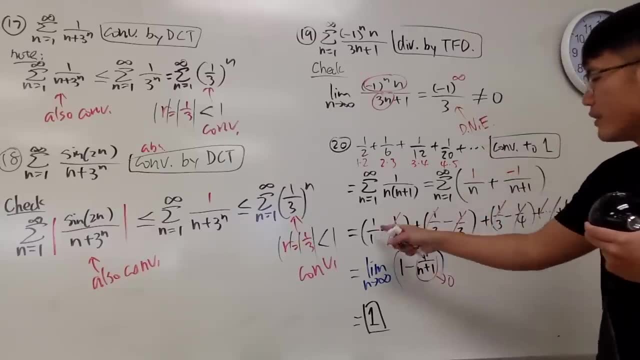 Very cool Telescoping series And another hint is that you see we have n and n plus 1. They're just off by one term. You have one term surviving, in the front, A number, And you'll see what I mean by that later on. We have a lot. 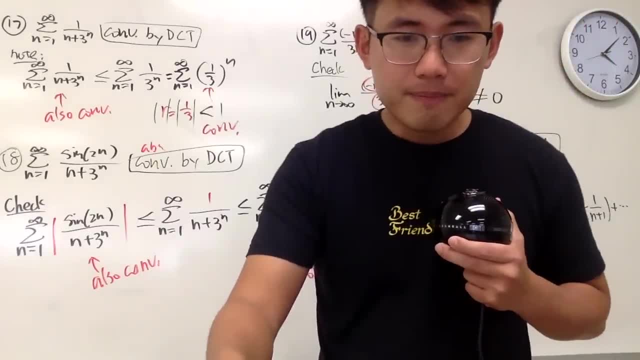 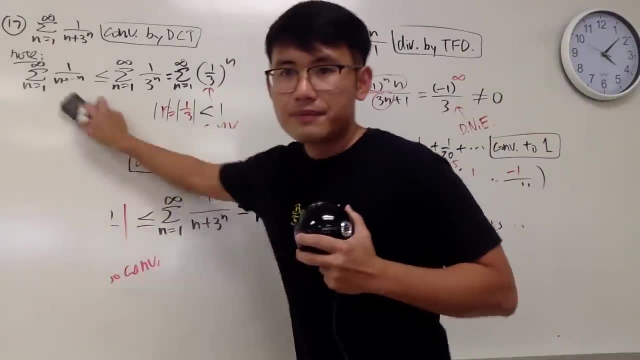 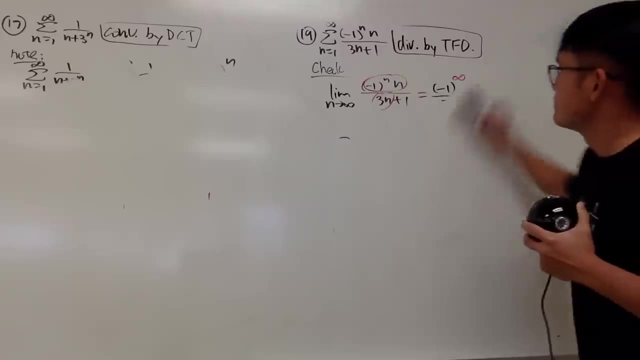 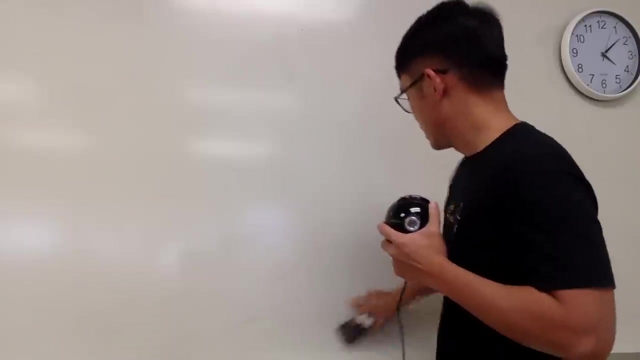 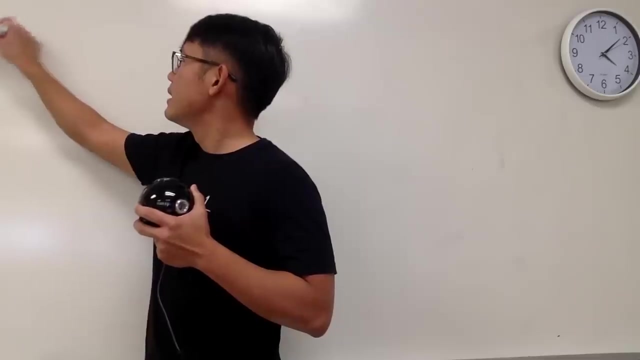 more coming, Well, not a lot more. Hmm, Okay, okay, okay, okay, okay, okay. So take a look, and then now let's continue. Let's see Number 21, right here. So here we have the sum as: 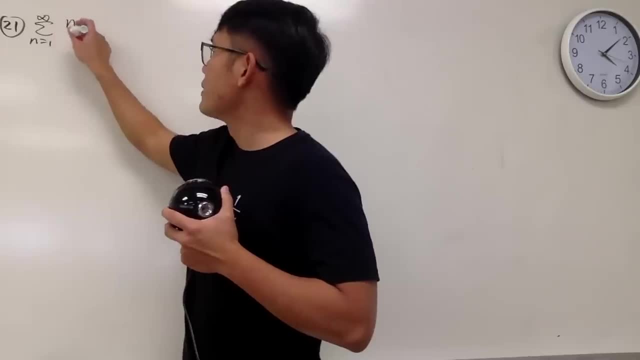 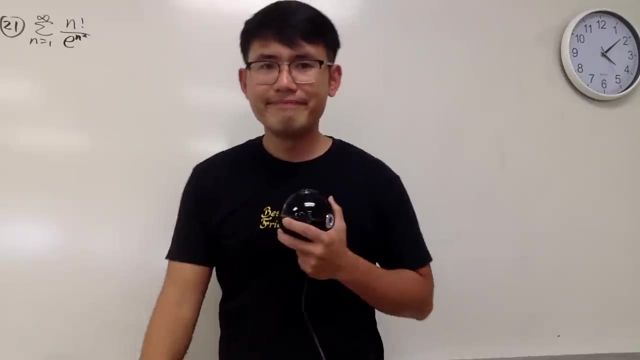 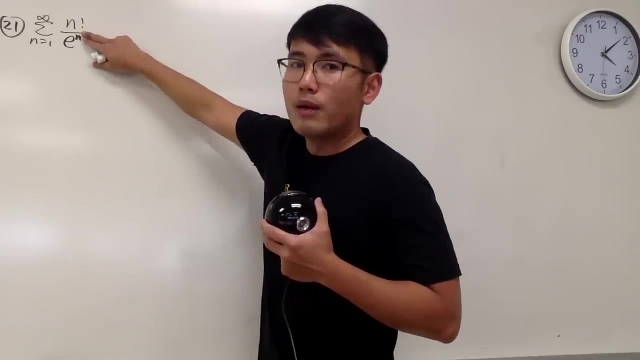 n goes from 1 to infinity And we have n factorial over n. I mean e to the n squared power. Hmm, Technically again, by the least n factorial is actually bigger than e to the n's power. But 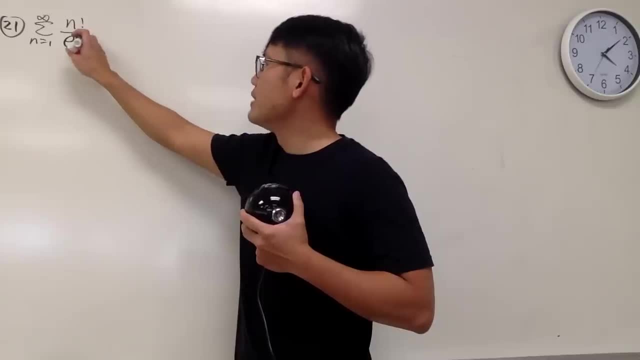 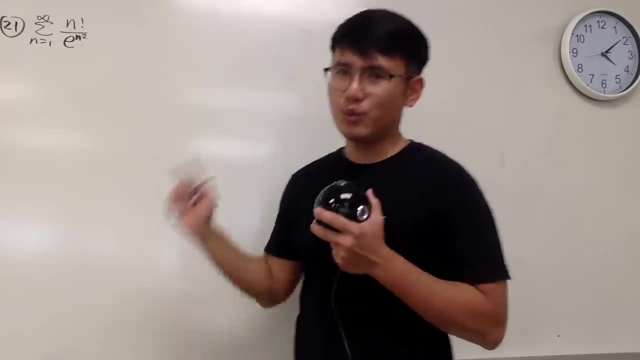 here we have another square. So, hmm, interesting, interesting, interesting. What should we do? Let's give the ratio test a try, because we have the factorial being involved. So this is the check that we are going to go through. 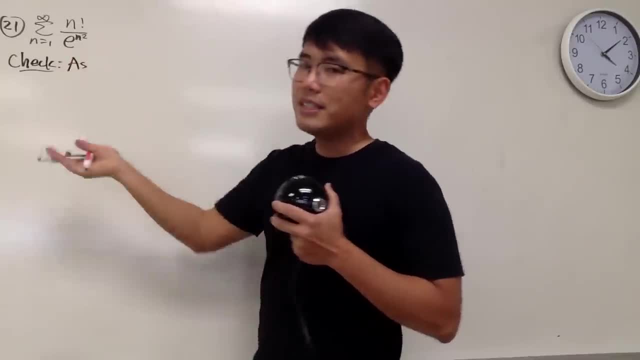 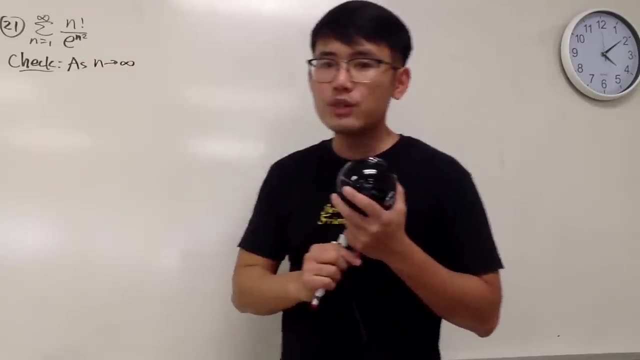 Again, let's write down the check. And now anything besides the test for divergence I will just put on as n goes to infinity And for the ratio test. first we are going to write down the absolute value and then the first term. right here is just: 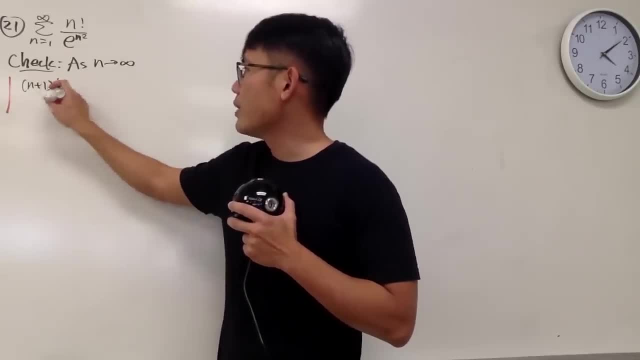 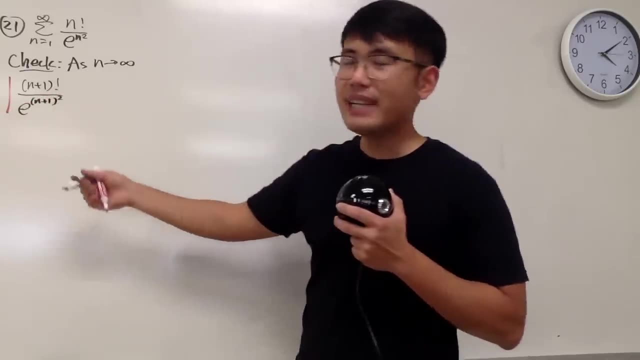 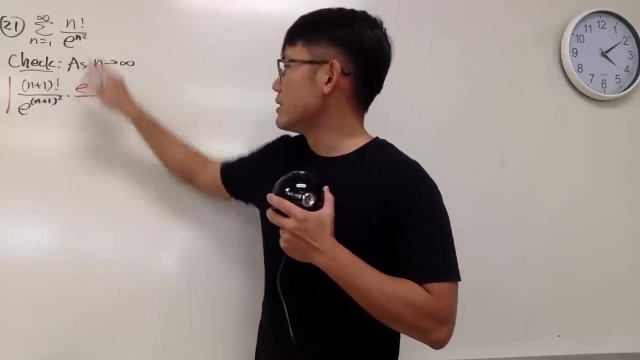 n plus 1, and then we have the factorial over e to the n plus 1, squared like that, Right. And then we multiply by the reciprocal of that, namely e to the n squared over just the n factorial, like this: 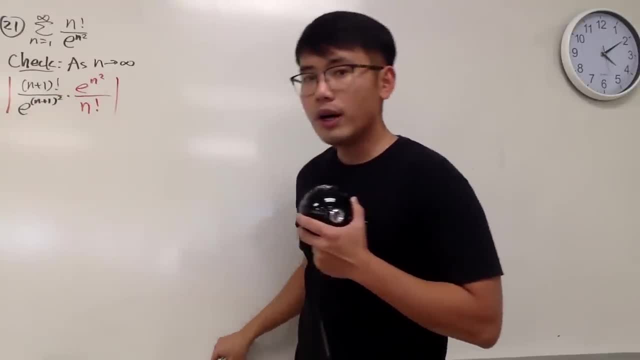 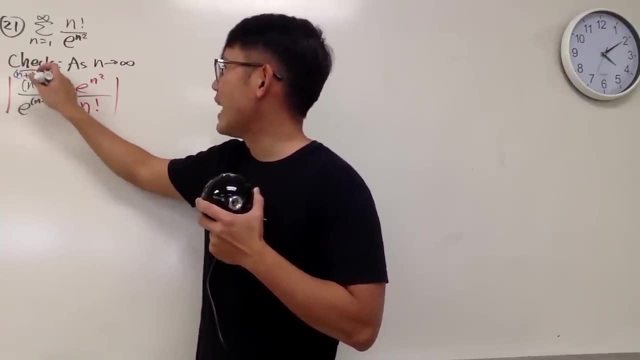 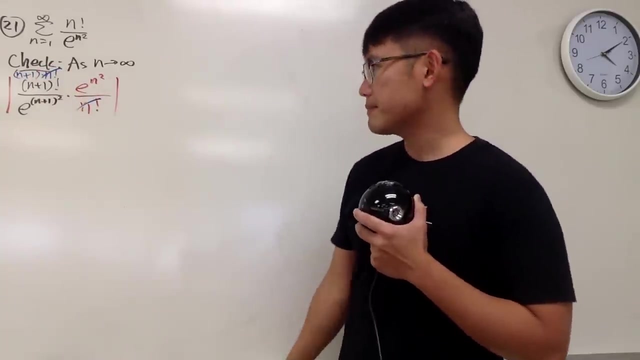 Now to break this down: we know n factorial plus n. we know n plus 1 factorial is just nicely equal to n plus 1 times n factorial. So this and that will be gone. Now let's look at that part. 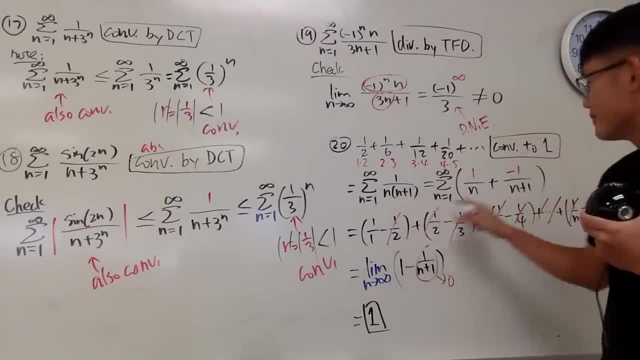 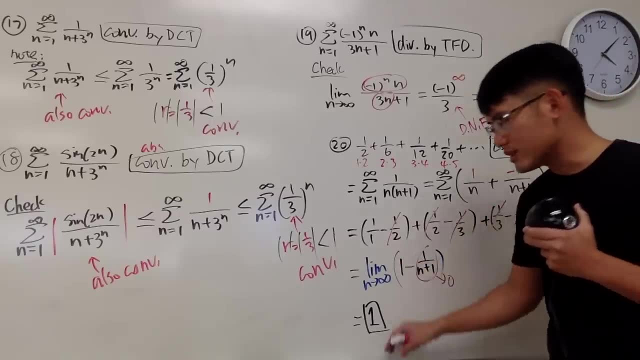 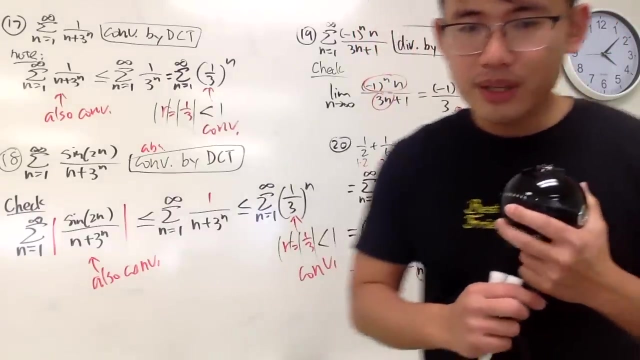 hint is that you see, we have n and n plus 1, they're just off by one term. you have one term surviving, in the front, a number, and you will see what I mean by that later on. we have a lot more coming. well, not a lot more that. hmm, okay, okay, okay, okay. 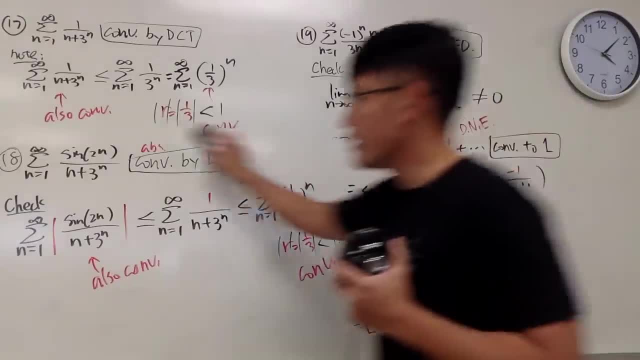 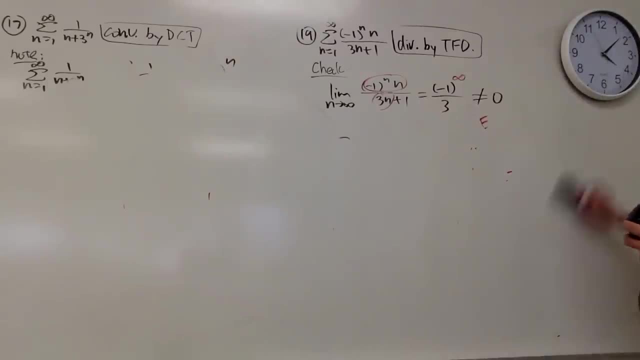 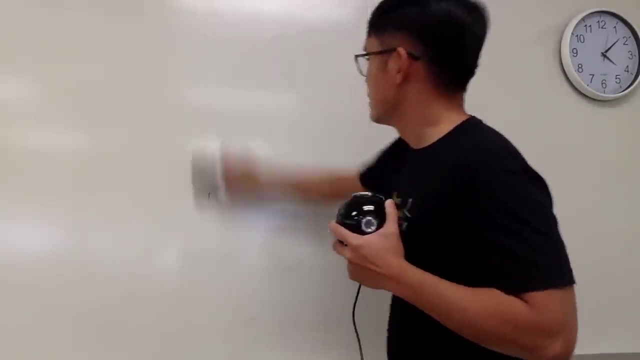 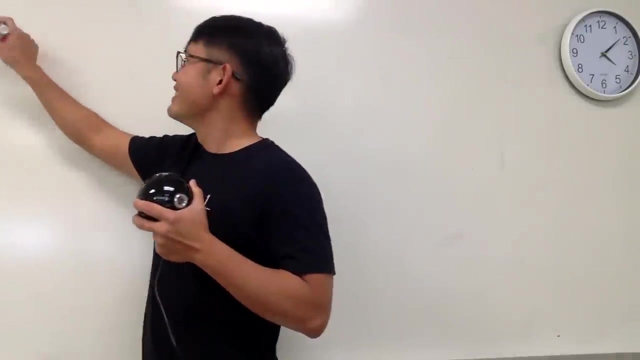 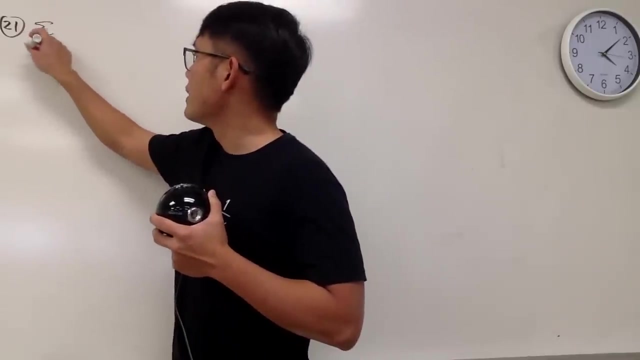 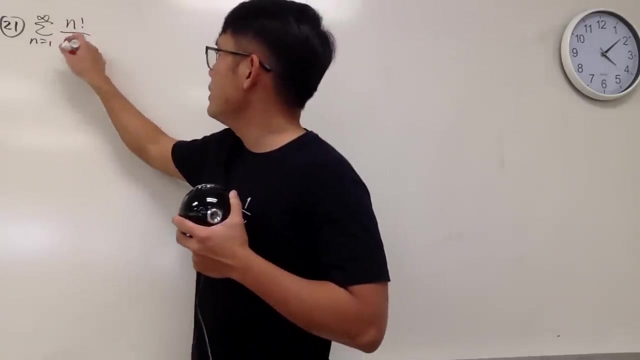 so take a look. and then now let's continue. let's see number 21, right here. so here we have the sum As n goes from 1 to infinity and we have n factorial over n. I mean e to the n square. 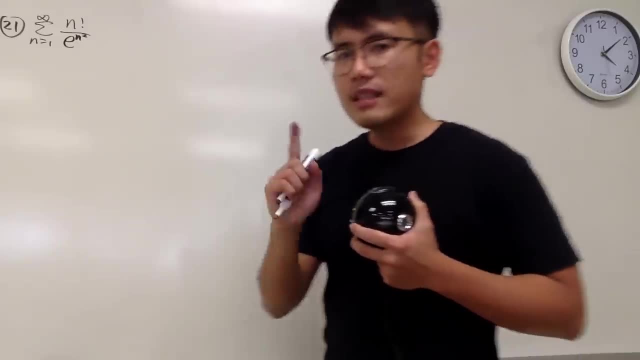 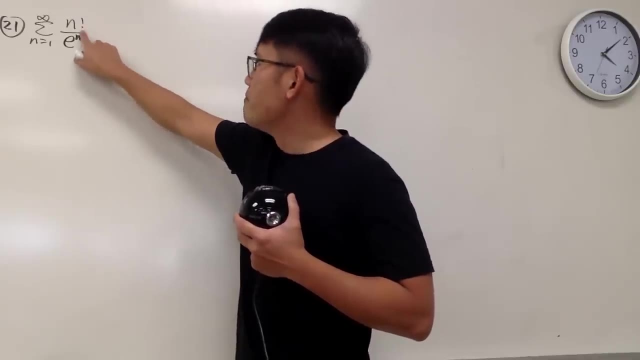 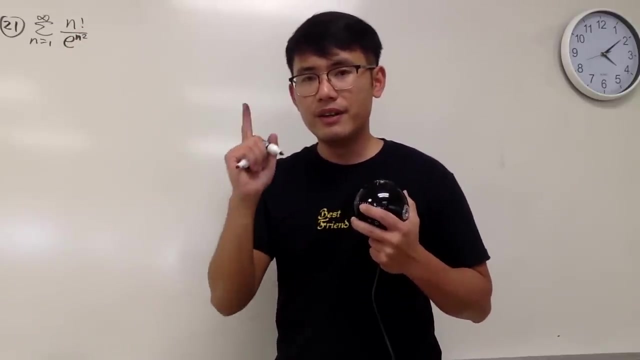 power. hmm, technically, again by the list, n factorial is actually bigger than e to the nth power. but here we have another square. so, hmm, interesting, interesting, interesting, interesting. what should we do? Let's give the ratio test a try, because we have the factorial. 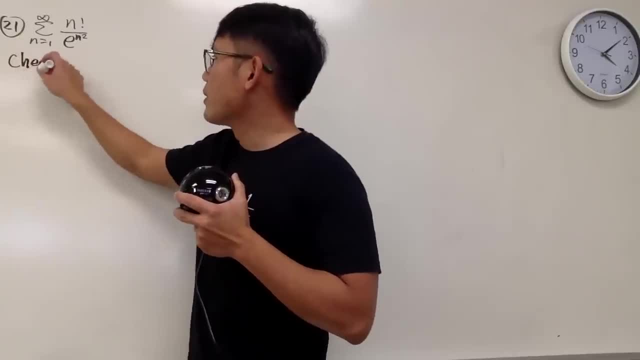 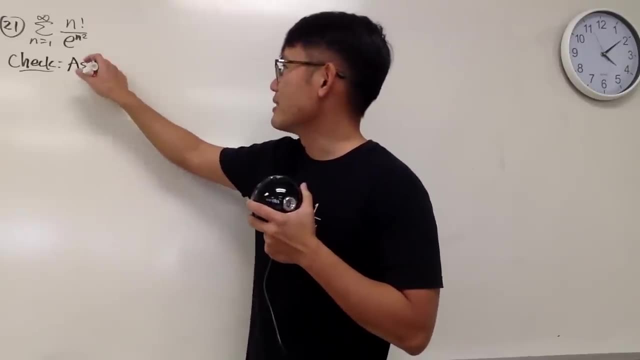 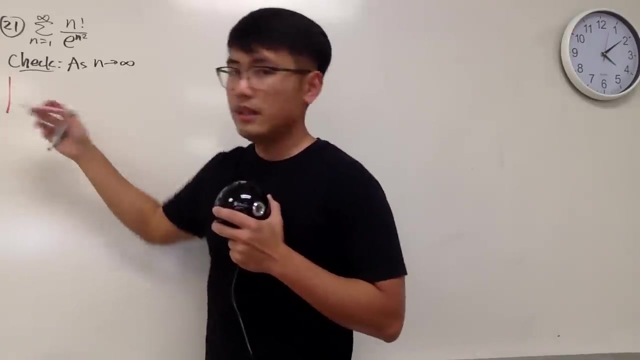 So this is the check that we are going to go through again. let's write down the check. and now, anything besides the test for divergence I will just put on as n goes to infinity- and for the ratio test. first we are going to write down the absolute value and then 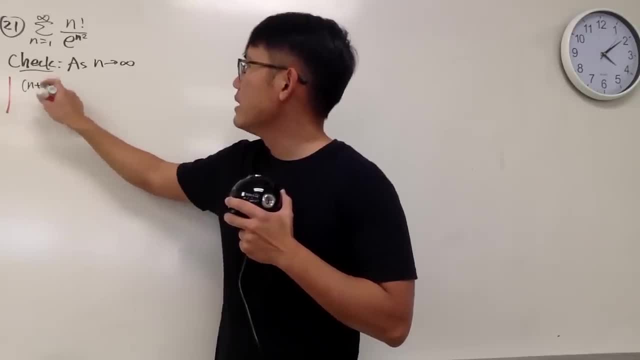 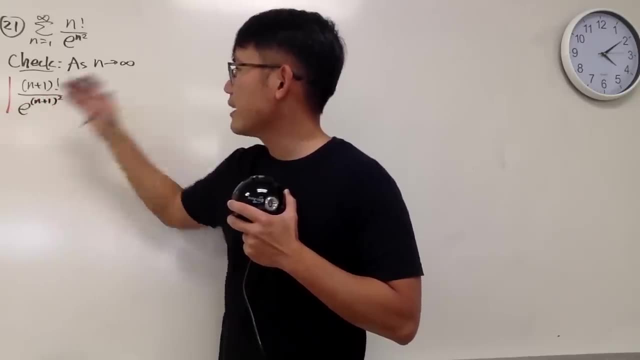 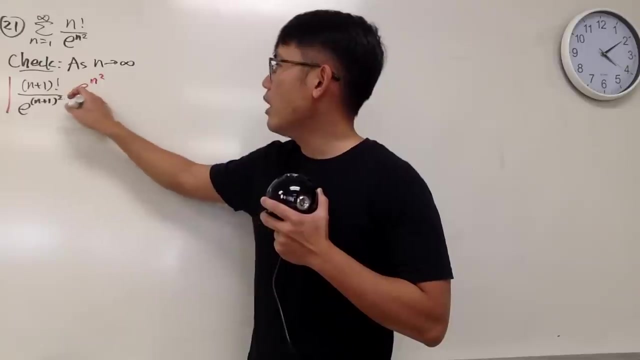 the first term right here is just n plus 1, and then we have the factorial over e to the n plus 1 square, like that. Okay, Okay, Like that Right. And then we multiply by the reciprocal of that, namely e to the n square over, just. 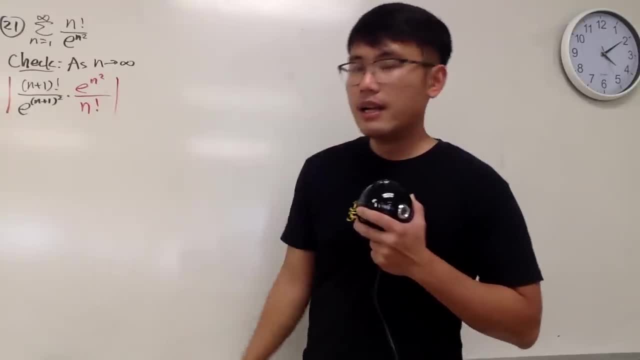 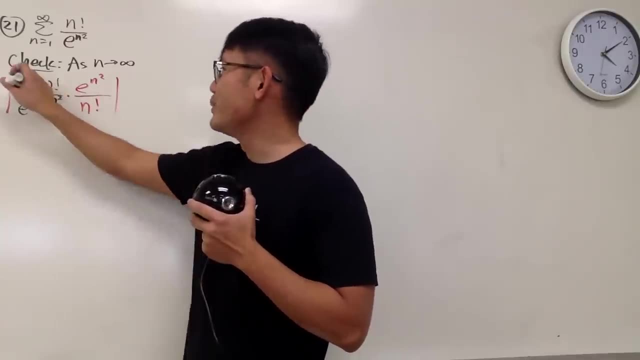 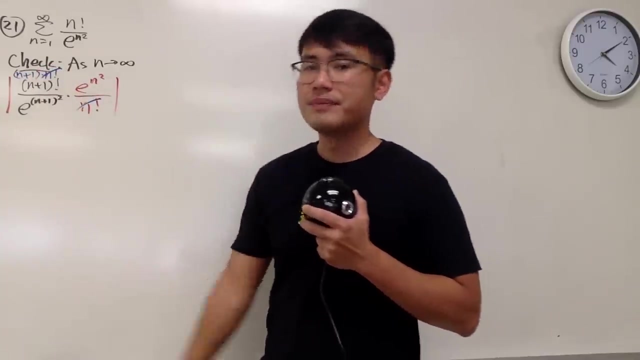 the n factorial. like this Now to break this down: we know n factorial plus n, we know n plus 1 factorial is just nicely equal to n plus 1 times n factorial. so this and that will be gone. Now let's look at that part. 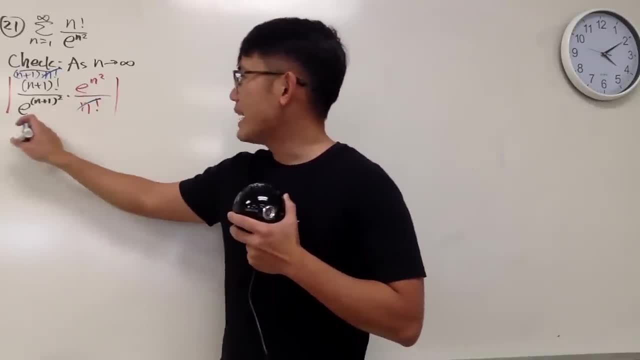 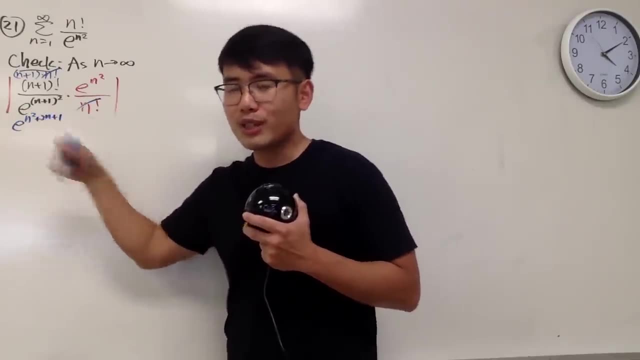 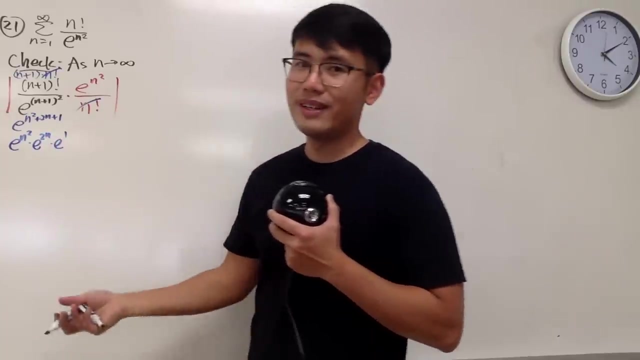 Hmm, Well, we expand that. In other words, we get e to the n? square plus 2n plus 1, and you are adding the powers right here so you can break them apart more. This is e to the n? square times, e to the 2n times, e to the first power and the beauty. 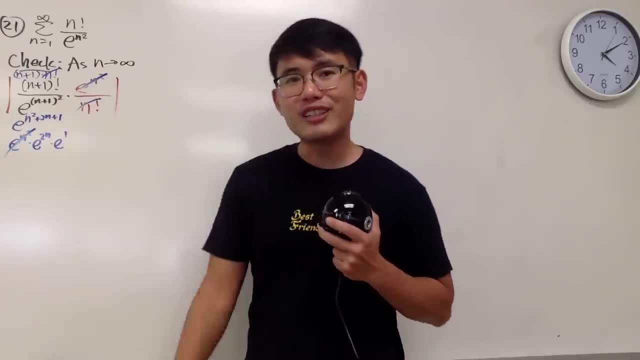 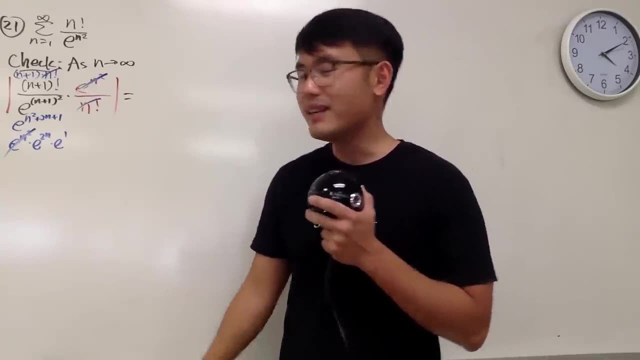 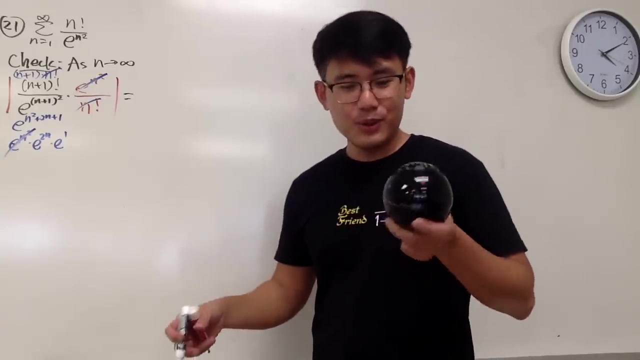 is that this and that cancel each other out as well. Now we see that this right here: everything is positive, so the absolute value doesn't matter. Oops, I should have done this like this, And now I didn't know, it was like that the whole time. 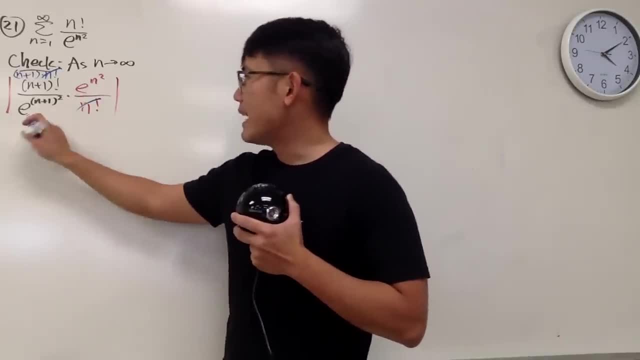 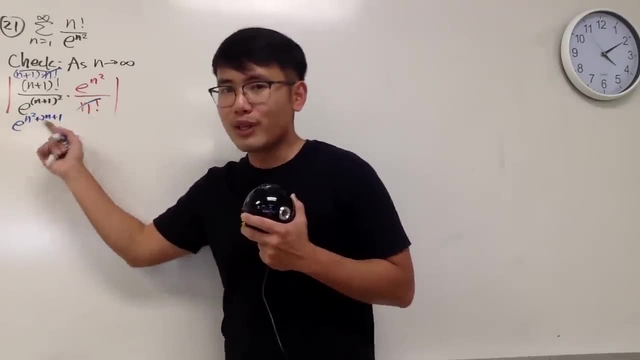 Hmm, well, we expand that. In other words, we get e to the n squared plus 2n plus 1, and you are adding the powers right here so you can break them apart more. This is e to the n squared times, e to the 2n. 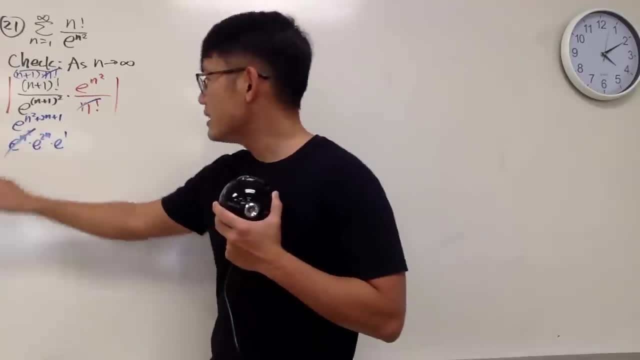 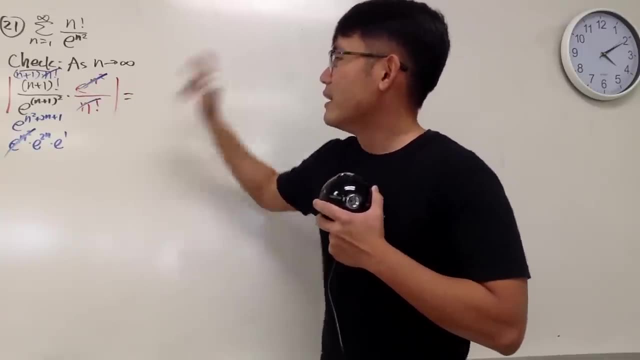 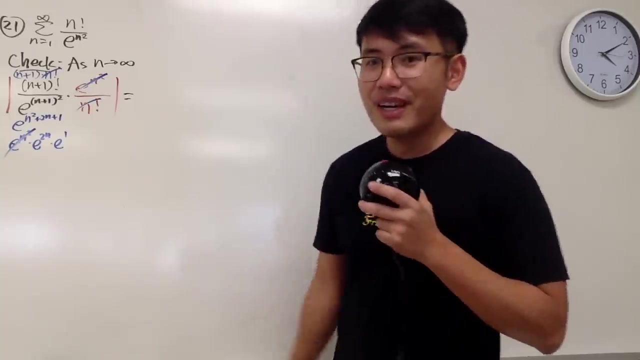 times e to the first power, And the beauty is that this and that cancel each other out as well. Now we see that this right here: everything is positive, so the absolute value doesn't matter, and we will just- oops, I should have done this like this. 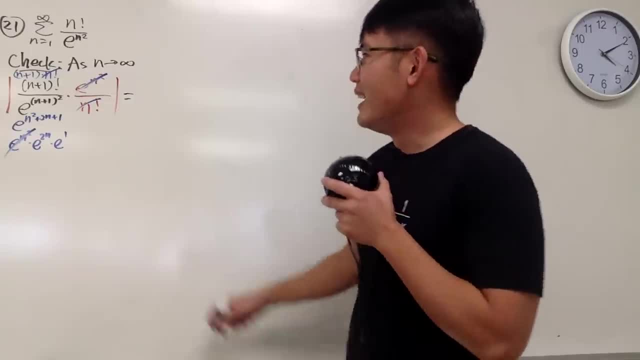 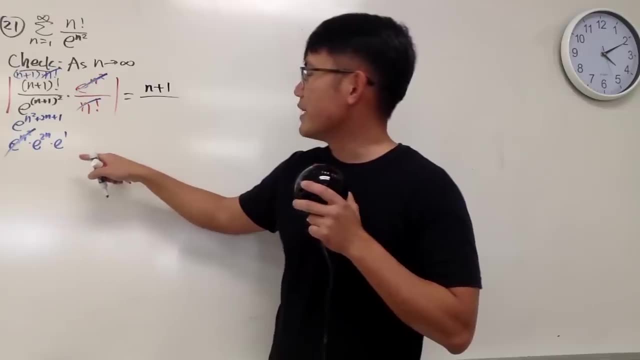 And now I didn't know, it was like that the whole time. And now we will just write down this right here on the top, which is n plus 1 over, and uh, the surviving part on the bottom is e to the 2n. 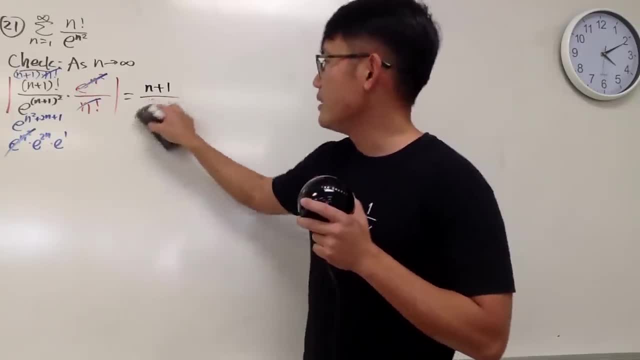 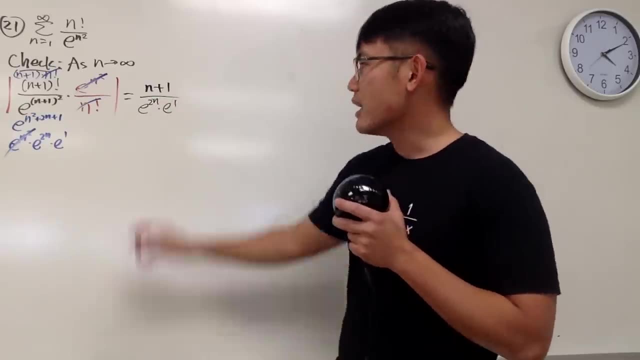 e to the 2n and then the e, right? So we just put down e to the 2n times e to the first power, like that, And check this out: On the top you have n to the p's power and on the bottom you have: 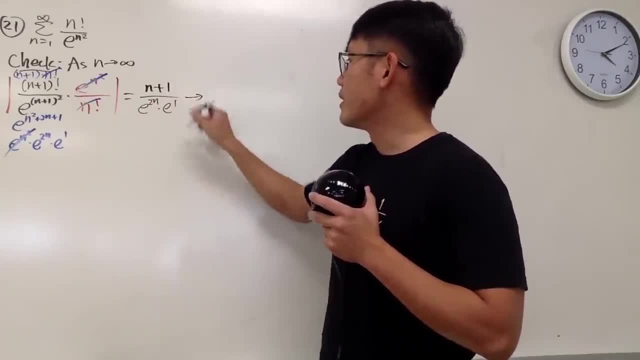 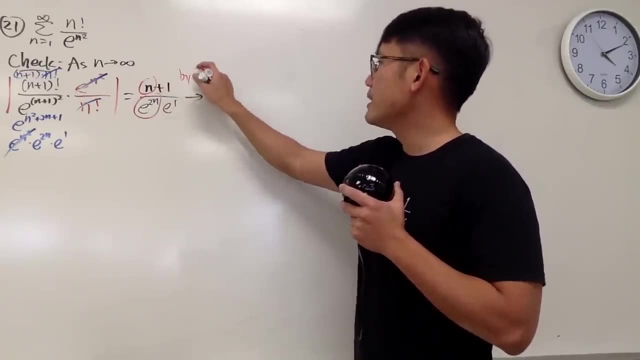 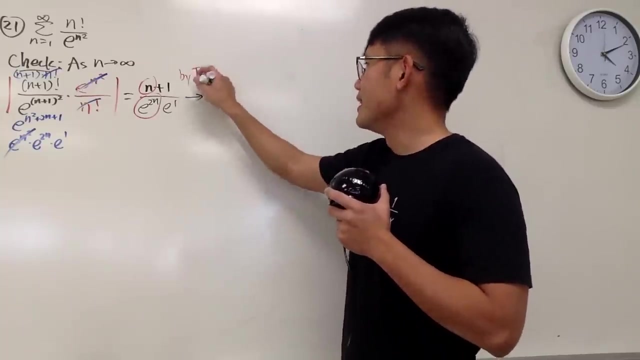 exponential. So by the list- you know this right here- goes to 0. And to do that you can just kind of circle this, circle that and you can also put down by the list And it seriously depends on your teacher, okay. So seriously, if your 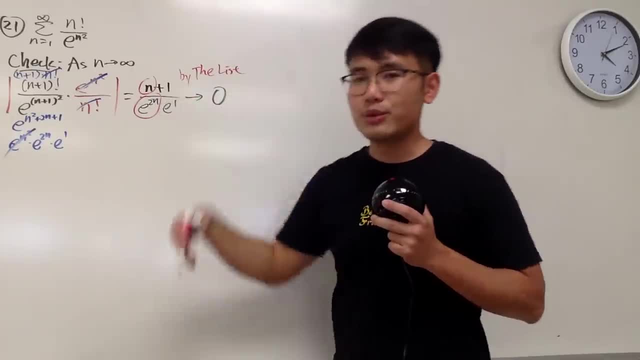 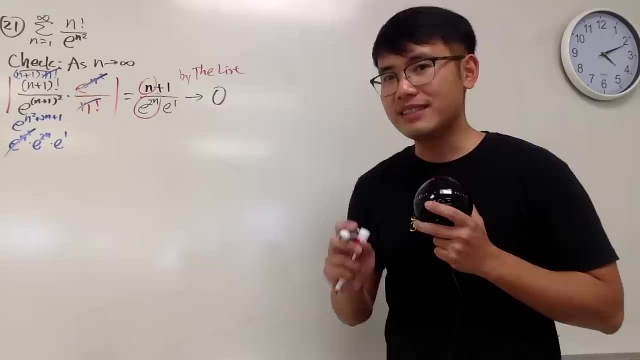 teacher is not cool with using the list, then just do. maybe change that to x and do Lapito's rule and all that. Alright, Now we did the limit. This is the real test and we get this is being 0.. Can we use 0?? 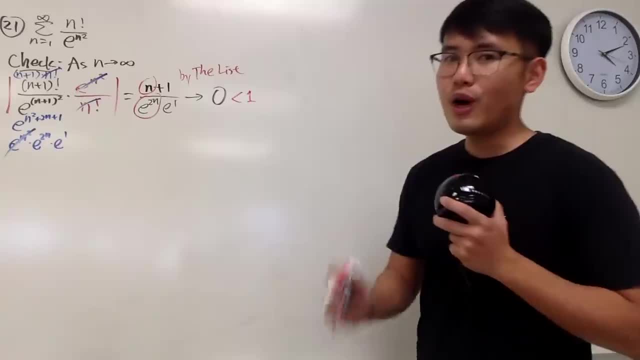 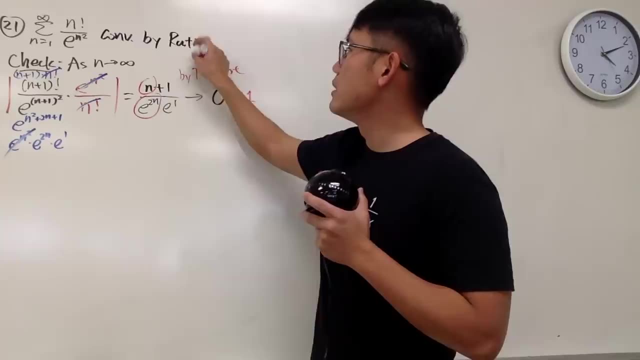 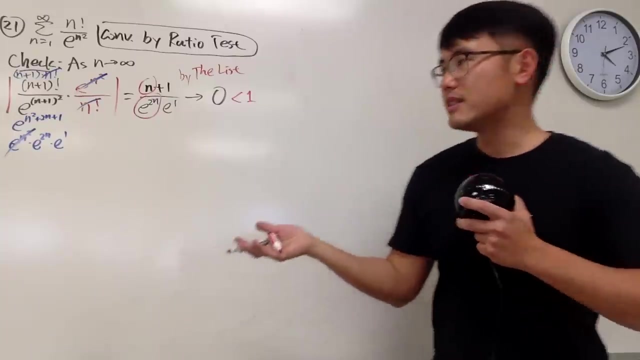 Yes, This right here is less than 1.. So we can conclude that this right here converges by the ratio test. Alright, So for the ratio test, it's. the idea is that you're comparing the next term with the current term, and 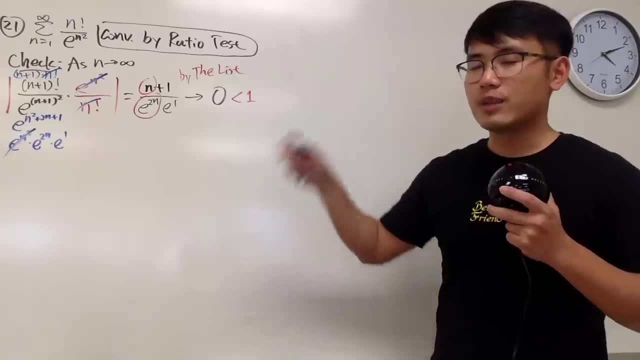 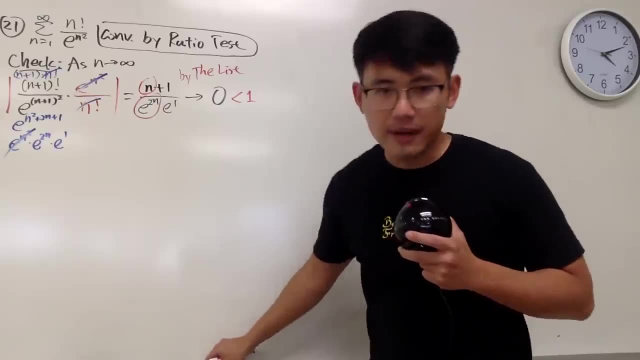 if the next term is strictly smaller, in the sense that the ratio is less than 1, you converge. That's the idea. So number 21 done, Okay, Now number 22.. Let's see number 22.. Here is the limit. 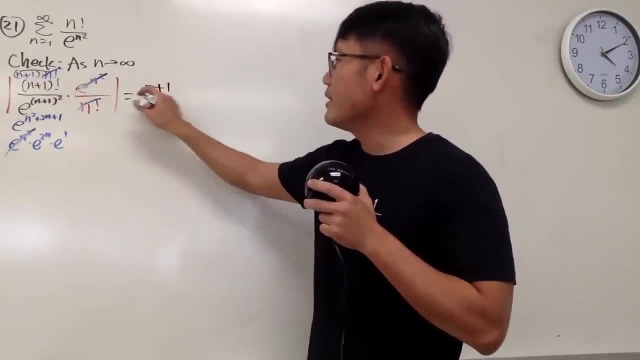 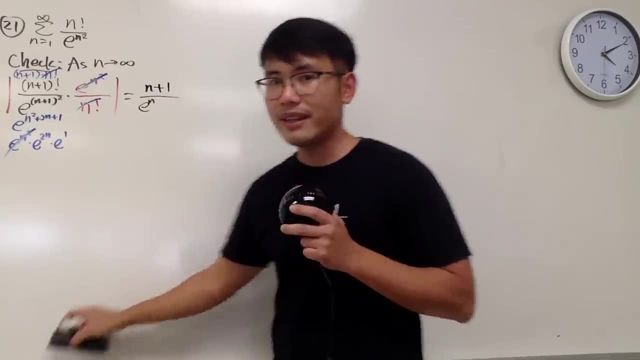 And now we will just write down this right here on the top, which is n plus 1 over, and the surviving part on the bottom is e to the 2n, e to the 2n and then the e. right, 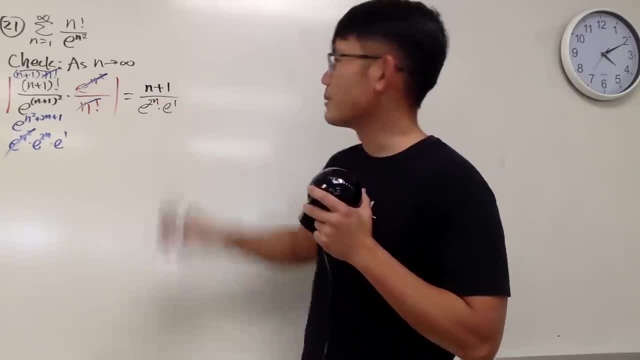 So we'll just put down e to the 2n times e to the first power, like that, And check this out: On the top you have n to the p's power And on the bottom you have n to the p's power. 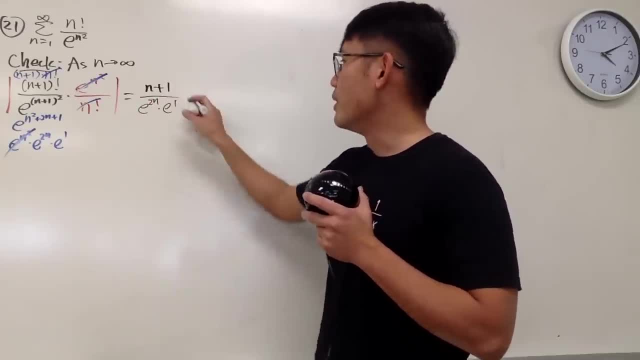 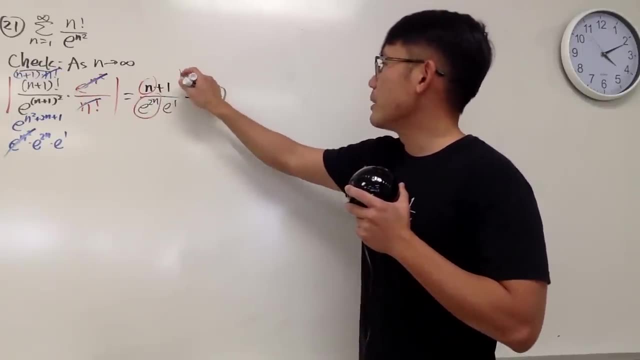 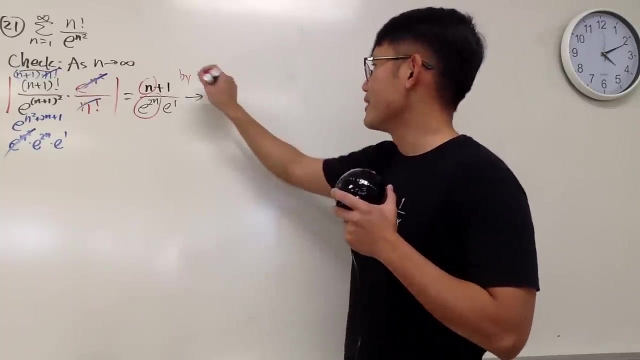 Okay, It's exponential. So by the list, you know this right here goes to zero And to do that you can just kind of circle this, circle that, and you can also put down by the list And it seriously depends on your teacher, okay. 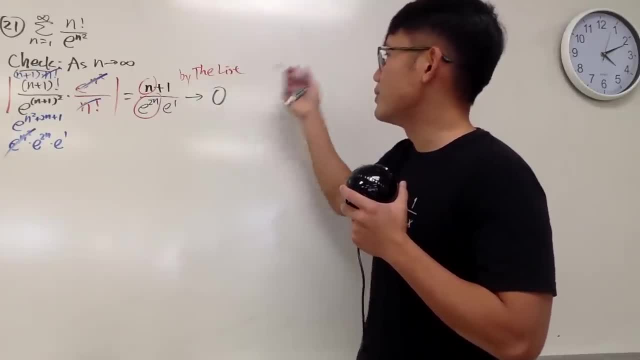 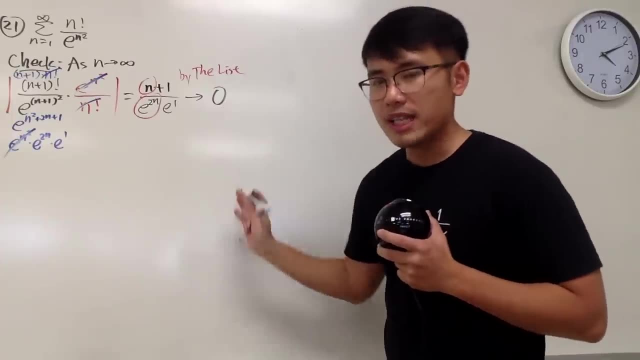 So seriously, if your teacher is not cool with using the list, then just do. maybe change that to x and do Lapito's rule and all that. All right, Now we did a limit. This is a real test And we get this is being zero. 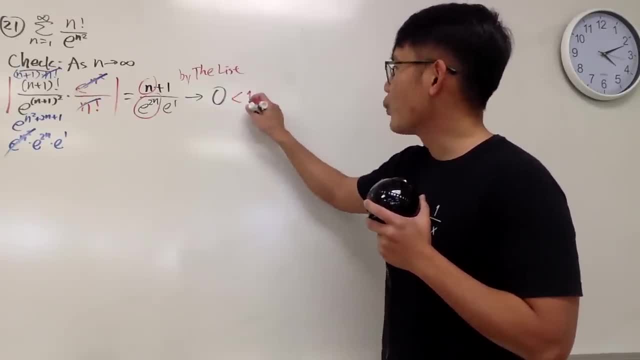 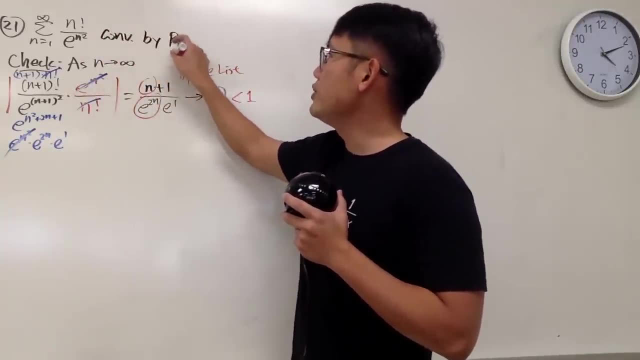 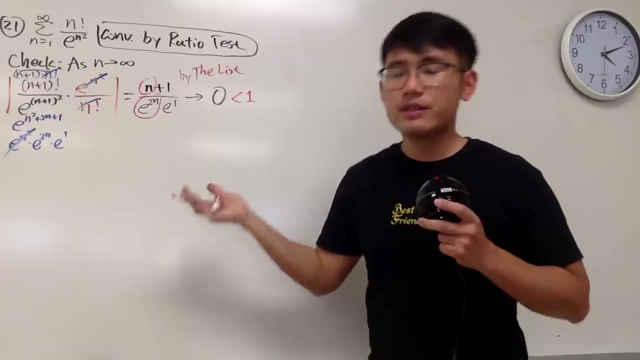 Can we use zero? Yes, This right here is less than 1.. So we can conclude that this right here converges by the ratio test, right? So for the ratio test, the idea is that you're comparing the next term with the current term. 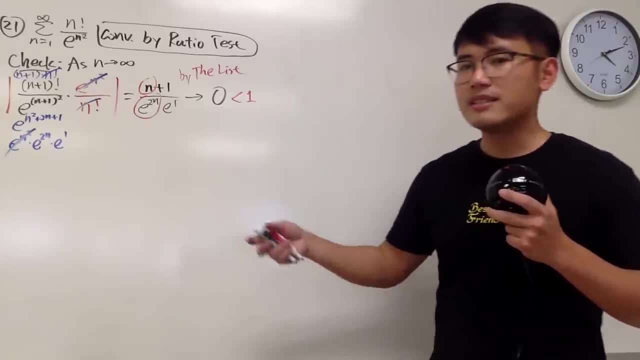 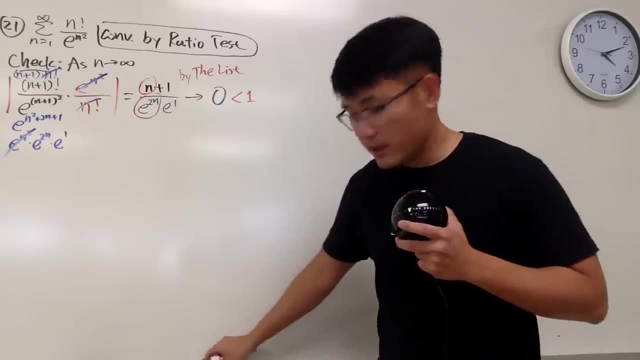 And if the next term is strictly smaller, in the sense that the ratio is less than 1, you'll converge. That's the idea. So number 21.. Done Okay, Now number 22.. Let's see Number 22.. 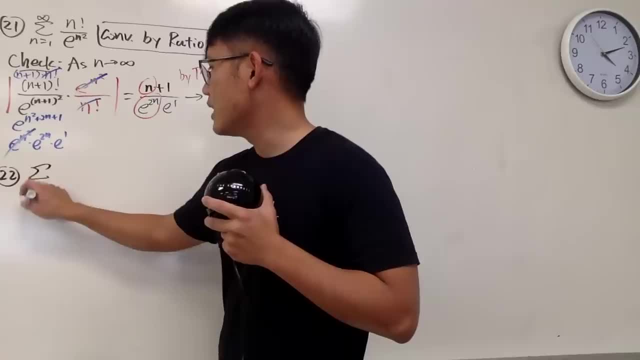 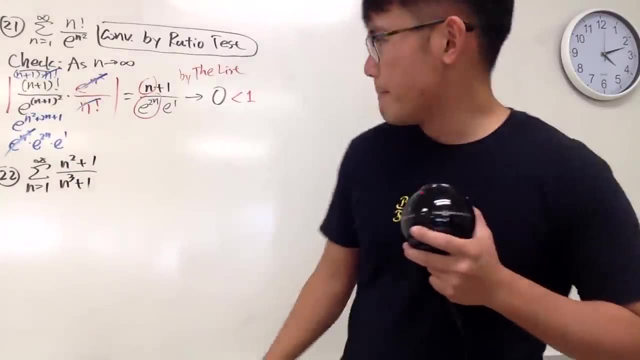 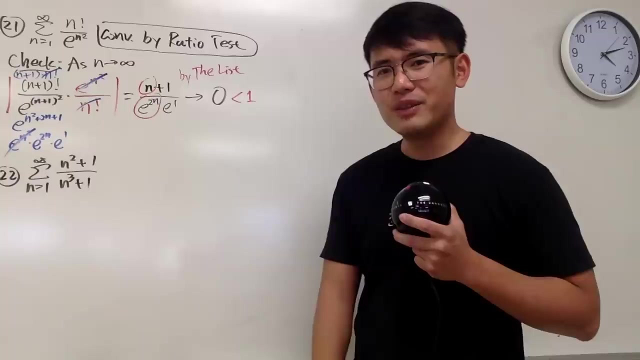 Here is the limit, as n goes from 1 to infinity, n squared plus 1 over n, to the third power plus 1.. If you cover everything, you just get 1 over n. Is this greater than 1 over n, though? 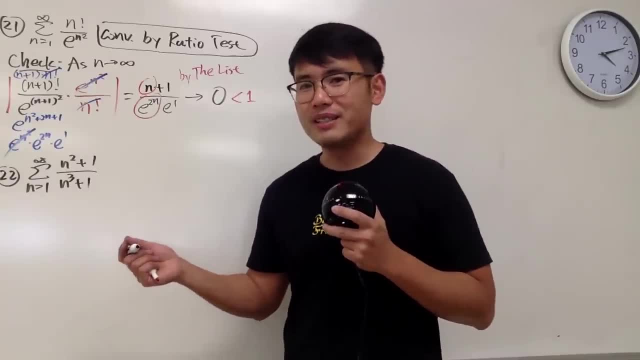 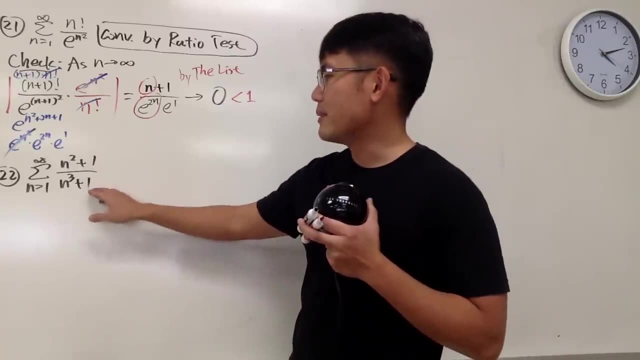 Hmm, You can try that. You can just try to do an inequality and all that. However, it's not generally easy to work out inequalities if you have something on top and then something being added on the bottom, unfortunately. So this is a better way to do it. 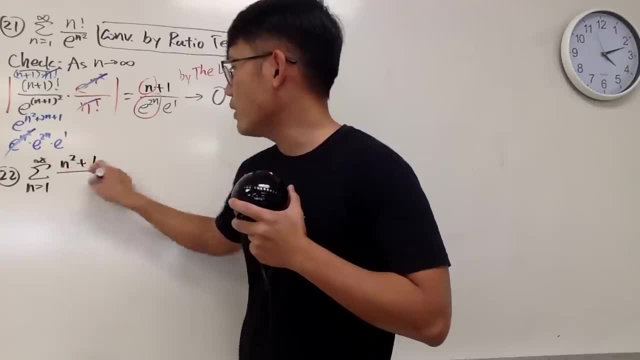 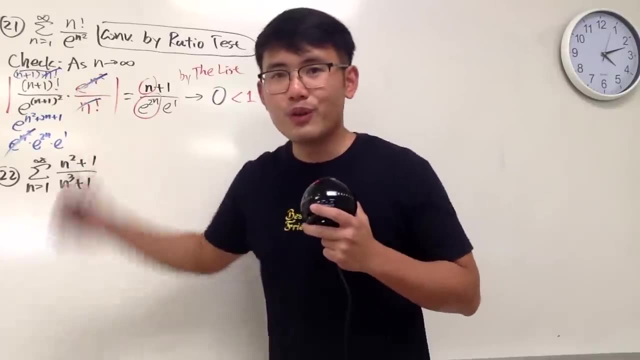 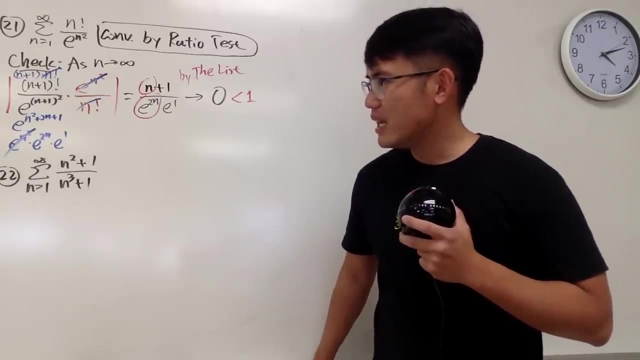 as n goes from 1 to infinity, n squared plus 1 over n, to the third power plus 1.. Hmm, If you cover everything, you just get 1 over n. Is this greater than 1 over n, though? Hmm? 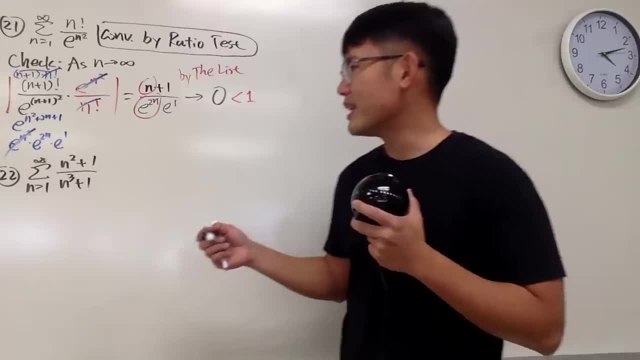 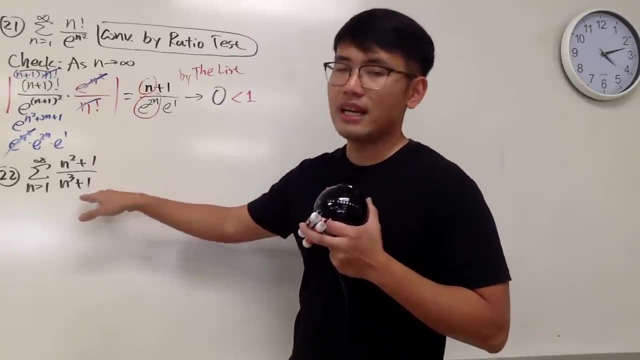 You can try that. You can just try to do like inequality and all that. However, it's not generally easy to work out inequalities if you have something on top and something being added on the bottom, Unfortunately, right. So this is a better way to do it. I will just do the limit. 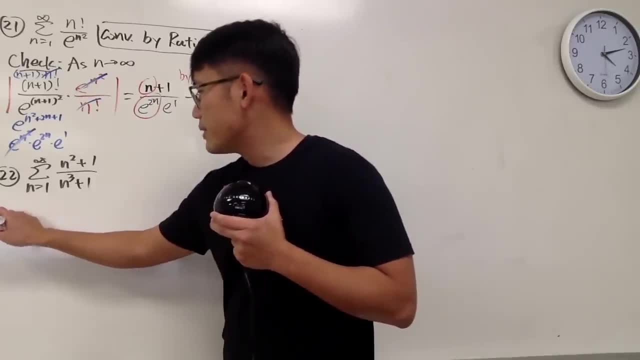 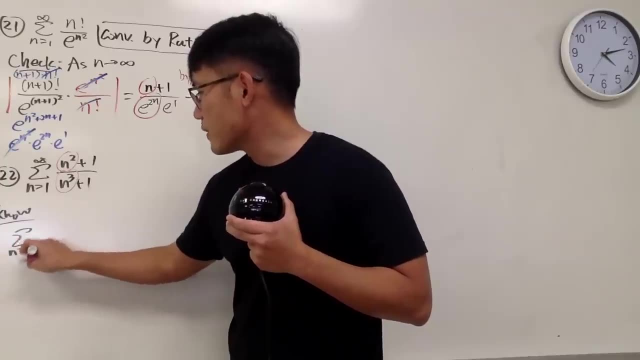 comparison test. So here we go, Let's put down what we know. And again, for what we know, just pick this and that. So this right here is the sum as n goes from 1 to infinity, n squared over, n to the third power. 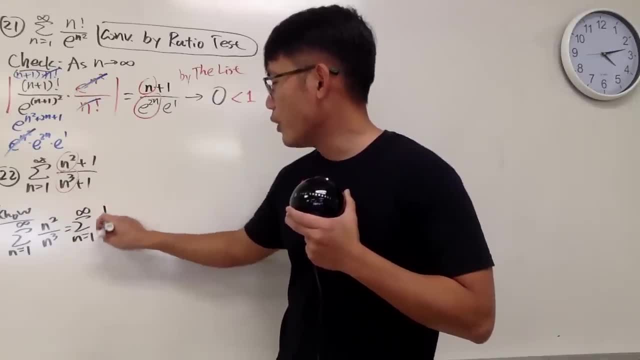 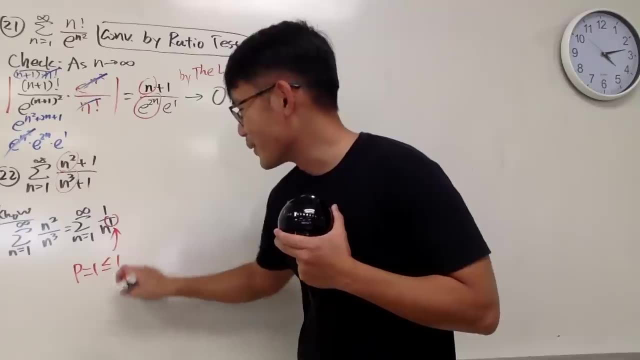 which is just the sum as n goes from 1 to infinity, 1 over n to the first power. This, right here, this is the first question that we did: p is 1, which is 10 to the equal to 1.. And this right here. 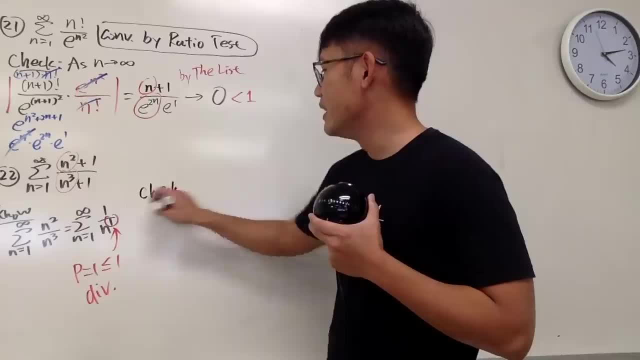 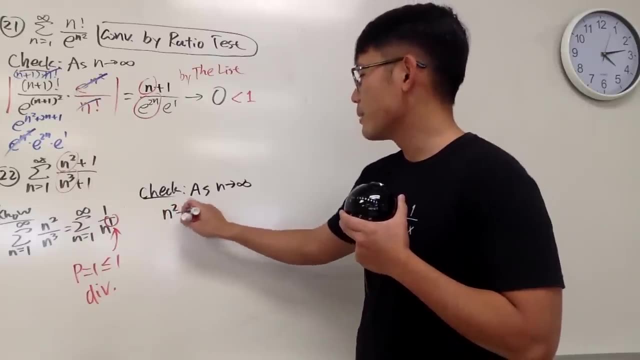 diverges. Secondly, we are going to check the limit And again I will just put down, as n goes to infinity, Put down the 1 that we want on the top, which is n squared plus 1 over n cubed plus 1, and 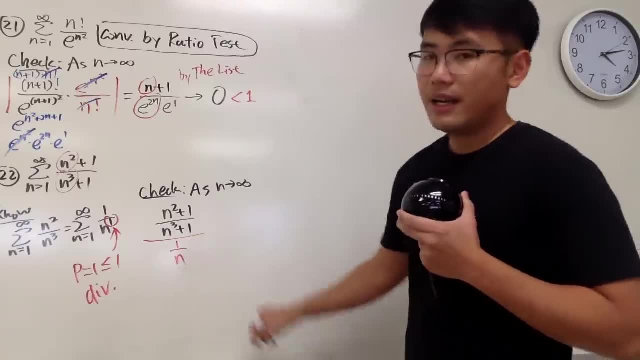 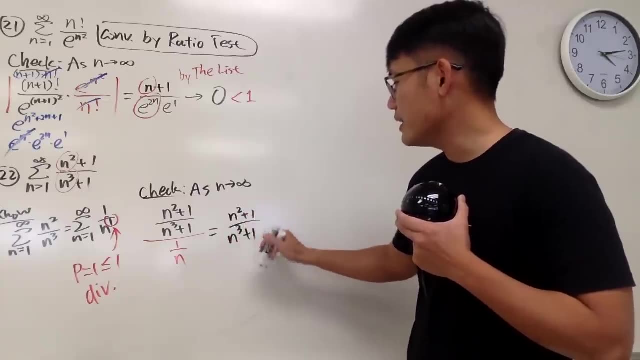 divided by the 1, that we know, which is 1 over n. And then we just flip that, This right here by doing algebra. we get n squared plus 1 over n, cubed plus 1 times n over 1.. And of course, put a little parenthesis. 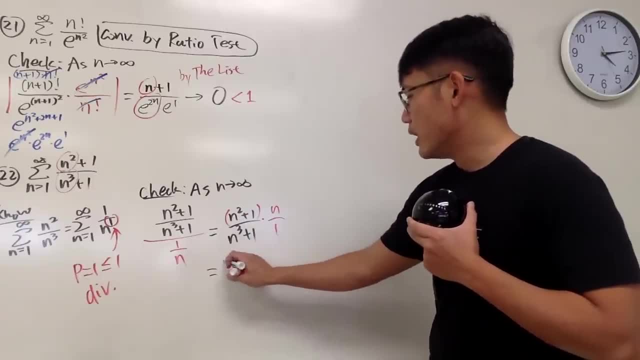 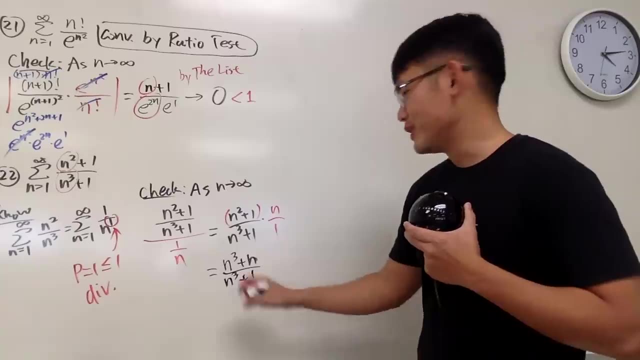 You can distribute this. You get this equal to n cubed plus n over n cubed plus 1.. And let's just do it this way: Circle this circle that or, if you would like, divide everybody by n to the third power. But you can see. 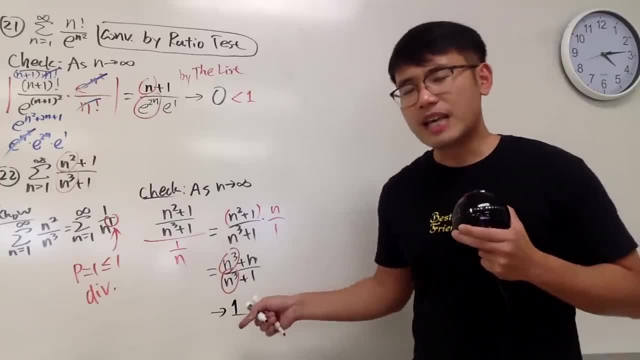 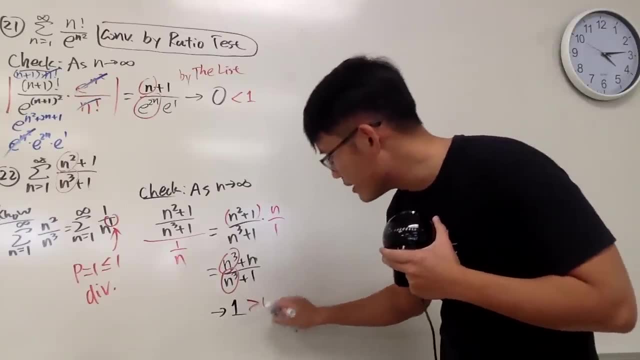 this right here: approaches 1.. Here can we use 1?? Yes, For the limit comparison test, 1 is good, because 1 is greater than 0.. 1 is greater than 0,, so we can use that alright. 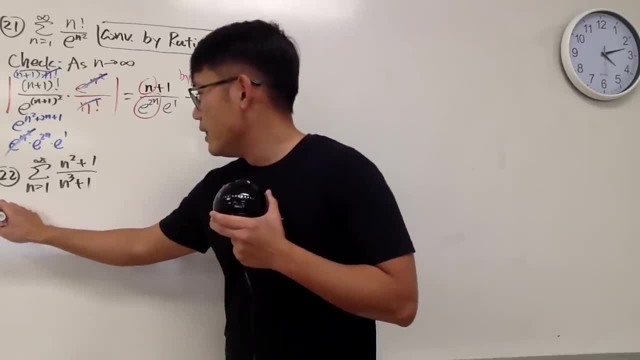 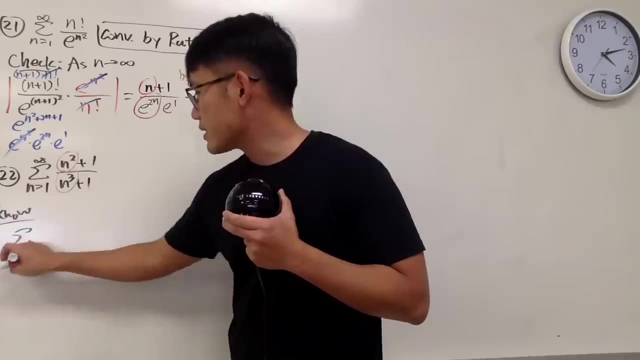 I will just do the limit comparison test. So here we go, Let's put down what we know. And again, for what we know, just pick this and that. So this, right here it's a sum as n goes from 1 to infinity, n squared over n to the third. 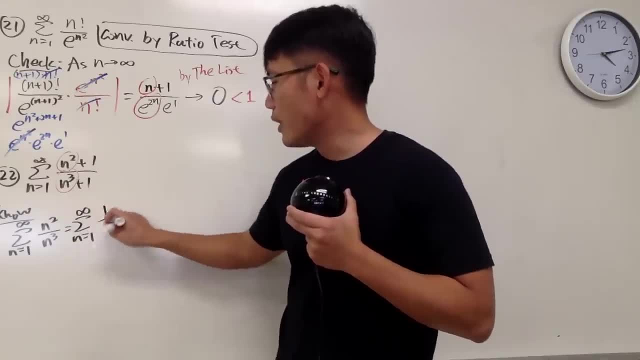 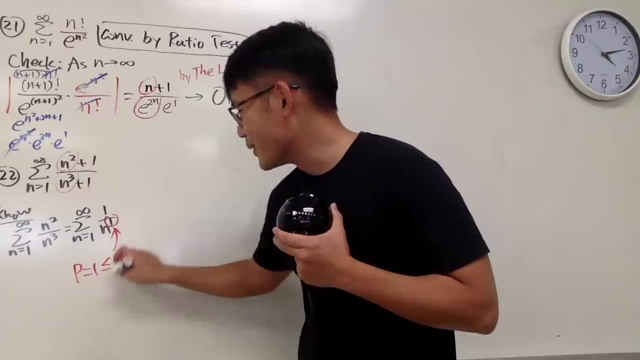 power. So this is the sum as n goes from 1 to infinity, 1 over n to the first power. This right here, this is the first question that we did- P is 1, which is 10 to the equal to 1.. 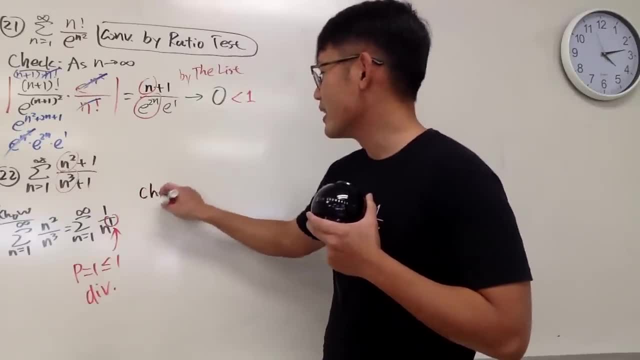 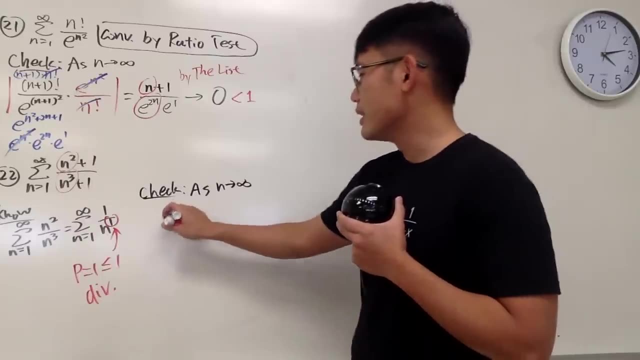 And this right here diverges. Secondly, we are going to check the limit And again I will just put down, as n goes to infinity, Put down the 1 that we want on the top, which is n squared plus 1 over n cubed plus 1, and 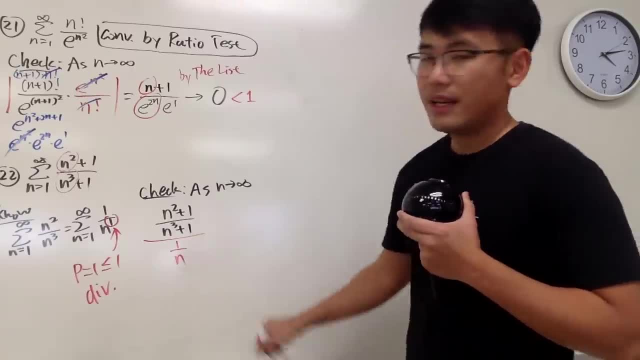 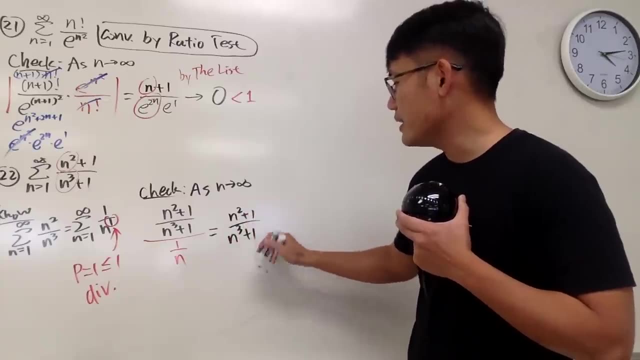 divided by the 1, that we know, which is 1 over n. And then we just flip that, This right here, by doing algebra: we get n squared plus 1 over n, cubed plus 1 times n over 1.. 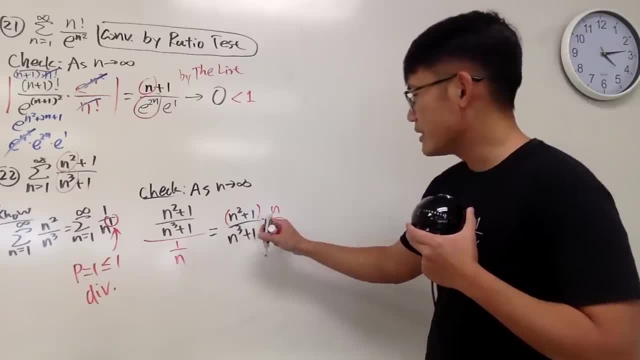 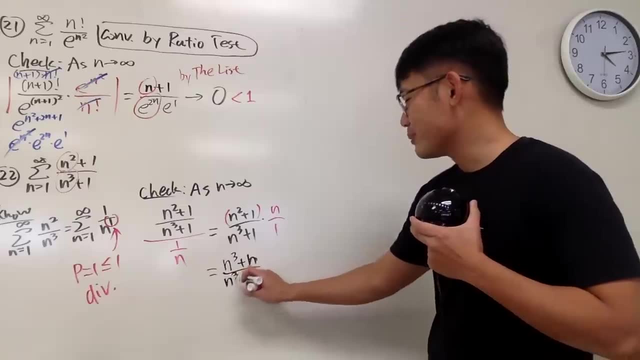 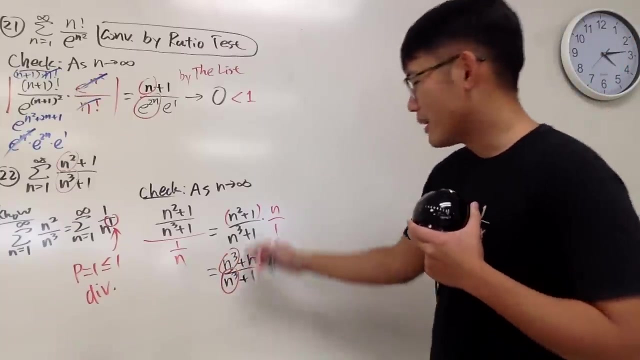 And then, of course, put a little parentheses. You can distribute this. You get this equal to n cubed plus n over n cubed plus 1.. And let's just do it this way: Circle this, circle that, Or, if you would like, divide everybody by n to the third power. 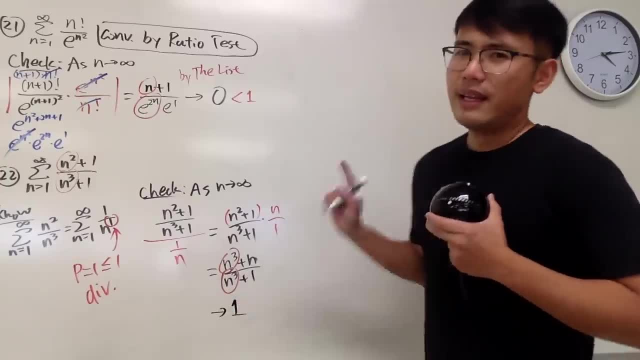 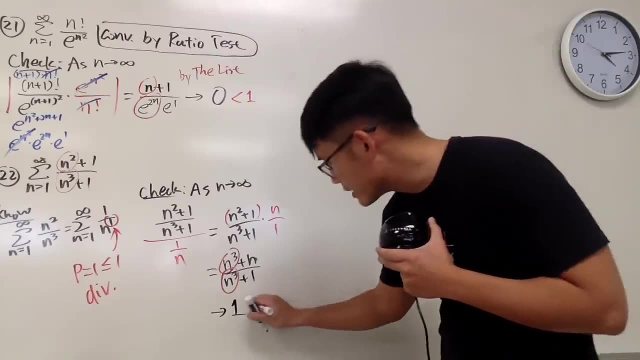 But you can see this right here. Approaches 1.. Here can we use 1?? Yes, For the limit comparison test, 1 is good, because 1 is greater than 0.. 1 is greater than 0,, so we can use that. 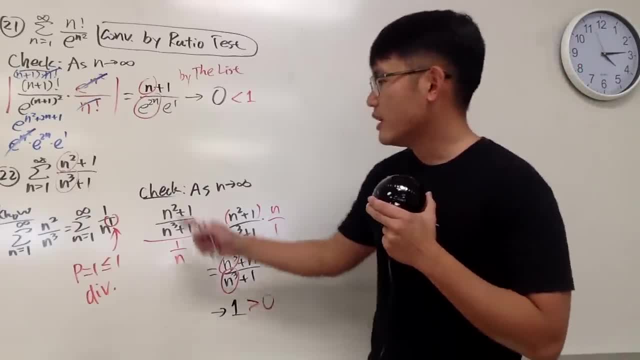 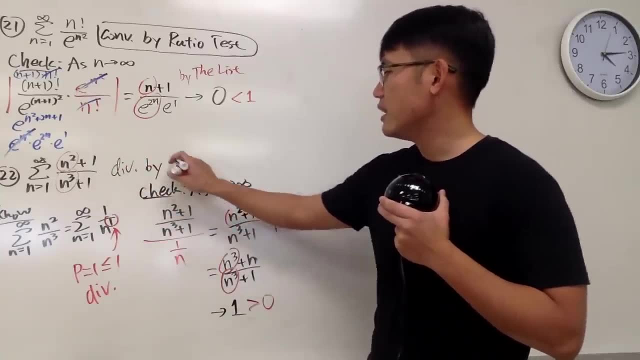 All right And we can draw a conclusion. They have the same conclusion, meaning that this right here also diverges. So I just put down: this right here Diverges by the limit comparison test, And then with that we are done. 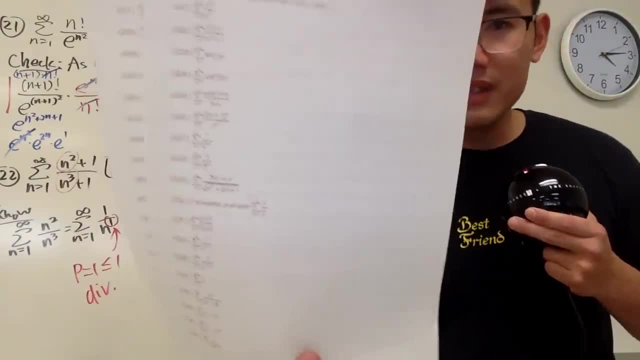 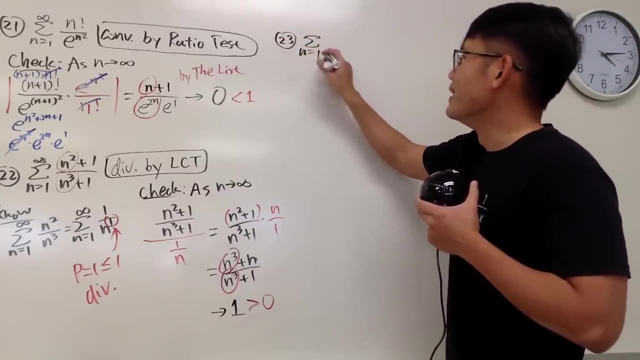 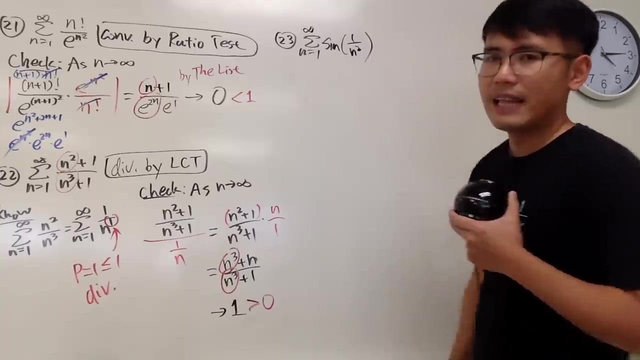 All right, Thank you. Next, we have the sine of 1 over n squared. So let's see Number 23.. So here we have the limit. No, no, no, no, no. Here we have the sum as n goes from 1 to infinity. sine of 1 over n squared. 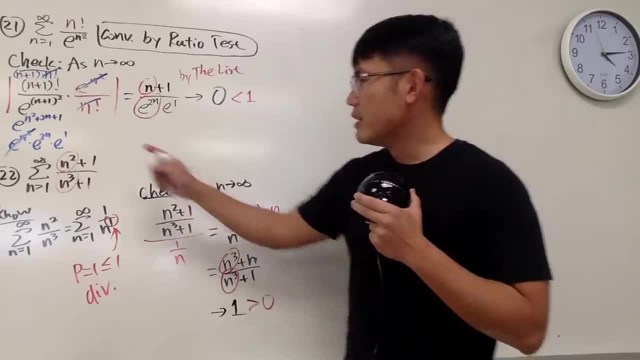 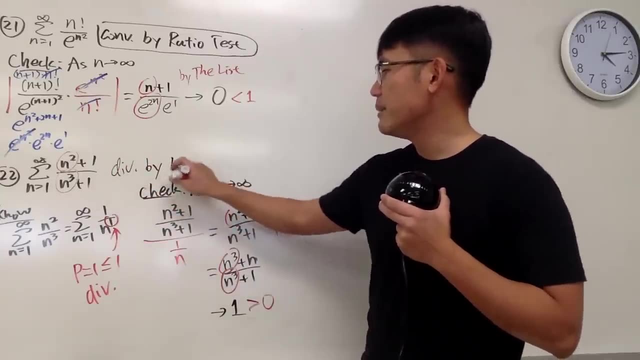 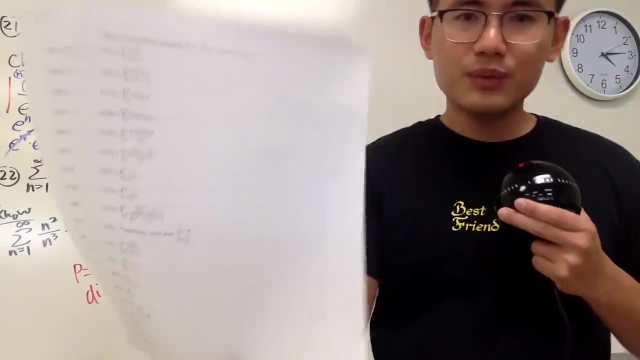 And we can draw a conclusion: They have the same conclusion, Meaning that this right here also diverges. So I just put down: this right here Diverges by the limit comparison test, And then with that we are done. Next we have: 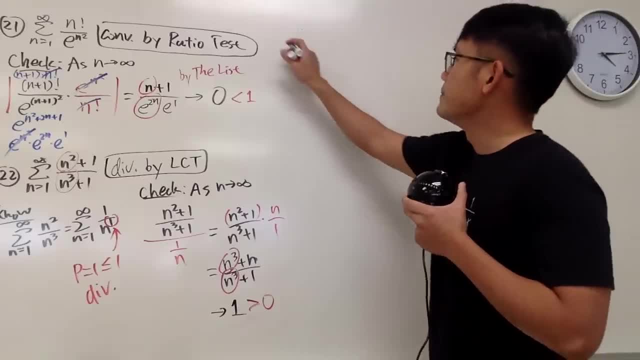 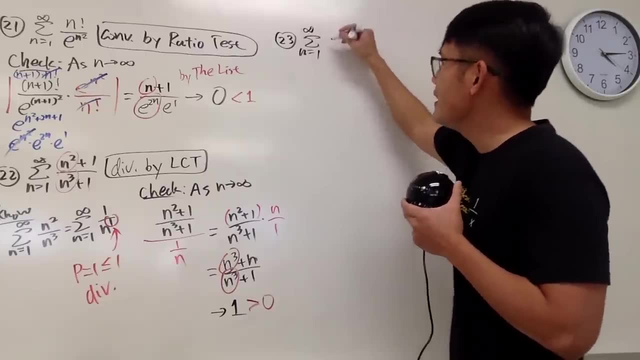 the sine of 1 over n squared. So let's see Number 23.. So here we have the limit. No, no, no, no, no. Here we have the sum as n goes from 1 to infinity sine of. 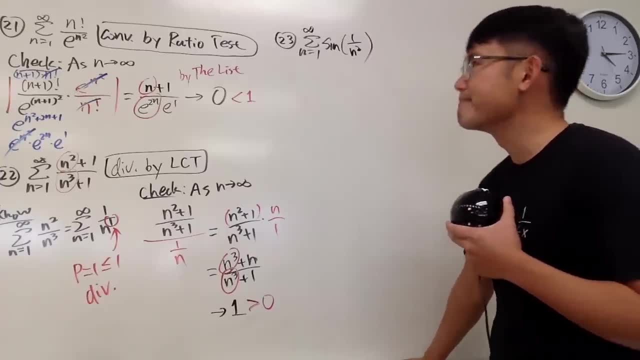 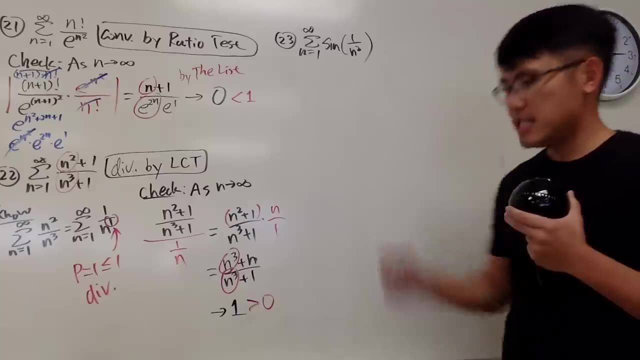 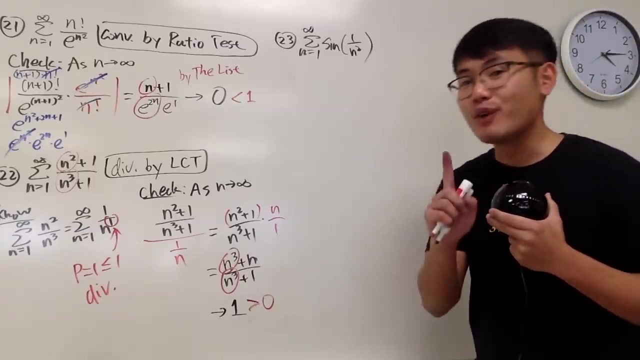 1 over n squared Like that. Hmm, Sine of 1 over n squared. Well, if you ignore the sine, that's good. First of all, let me tell you guys that everything is positive right here Again, okay, And. 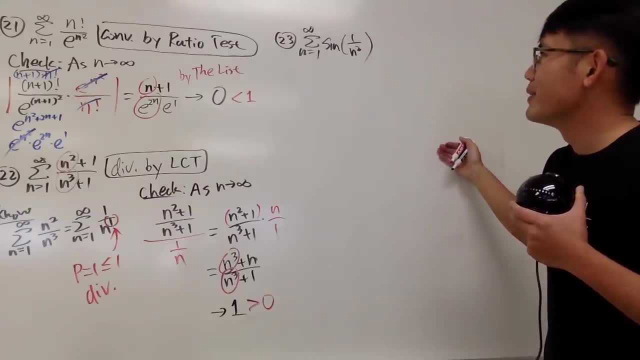 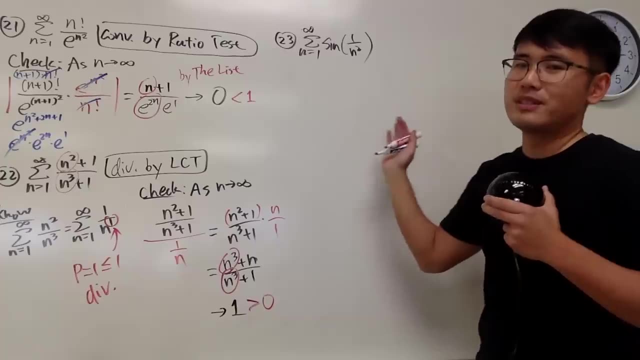 it's decreasing. If you want, you can maybe do direct comparison test, but I'm not sure about how this is compared to less than or equal to 1 over n squared. To be honest, I don't know. Usually it's hard. 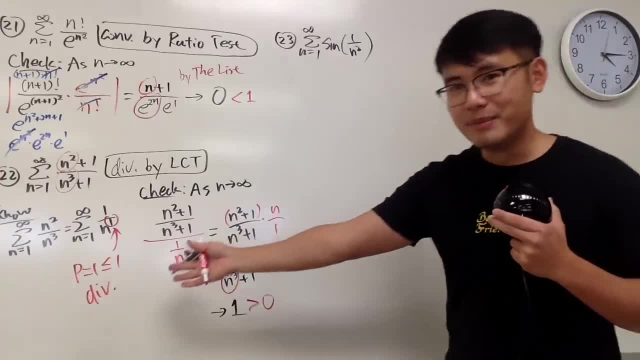 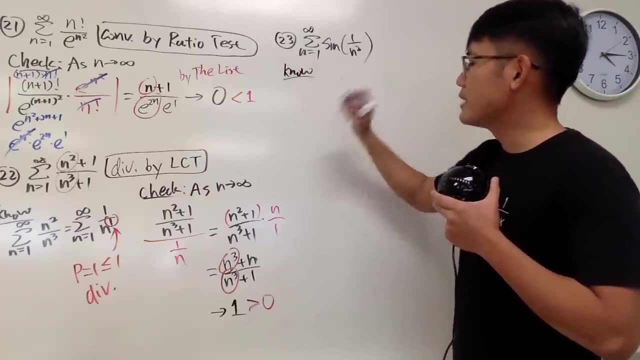 when you have a sine cosine and all that stuff. So again, let's try the limit comparison test. very nicely. So I will do that right here. I have the limit comparison test in my head, I'm going to use that. So this: 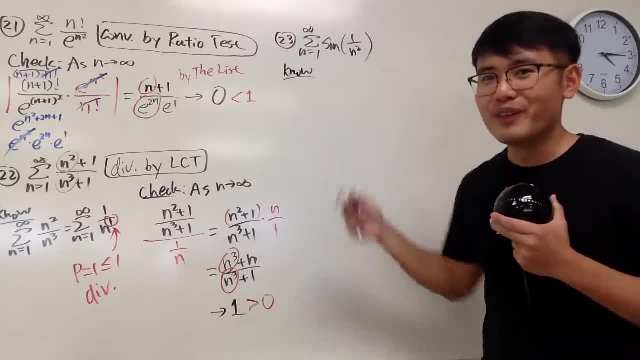 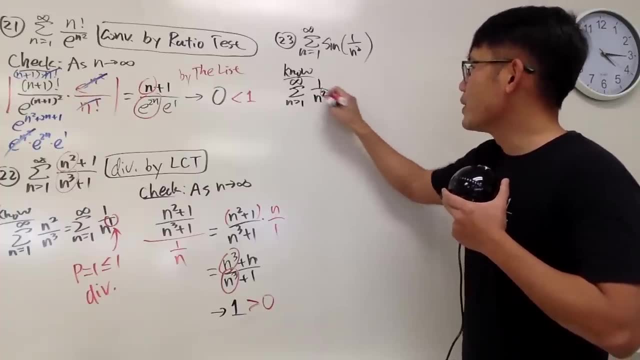 time. I'll just pick the p-series that we can see, which is 1 over n squared. So I'll just say: we know that the sum as n goes from 1 to infinity 1 over n squared. Here we go again. 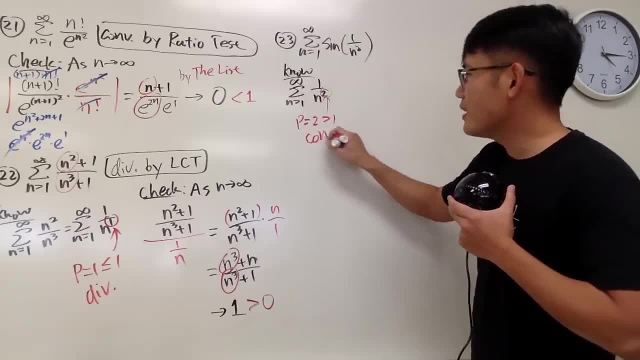 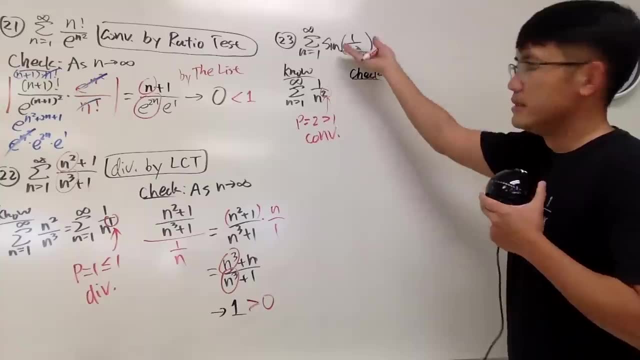 p is 2, which is greater than 1, which, right here, it converges. right Now we are going to check. this is what we know, right? So this is what we have. so let's just put this down right here. Namely, we'll. 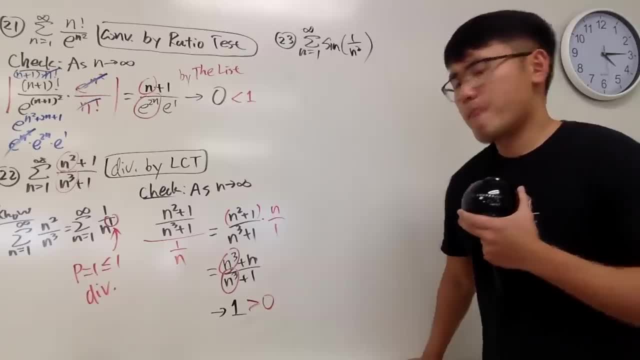 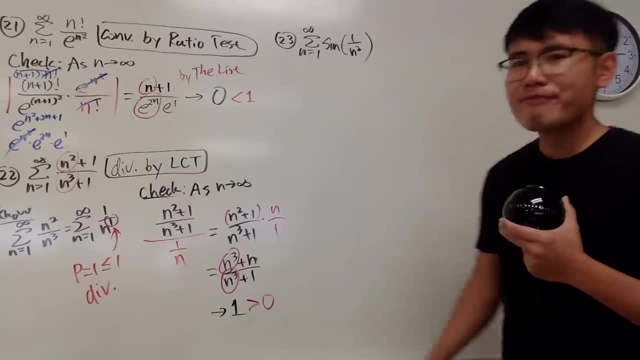 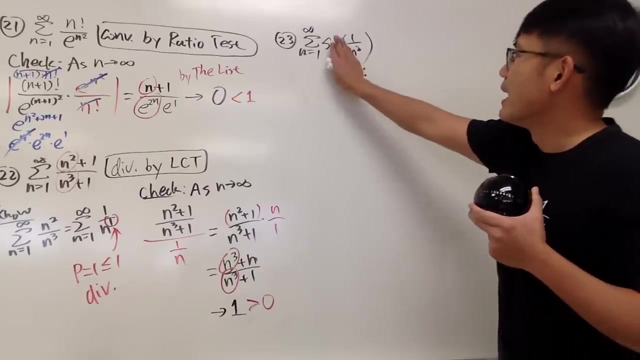 Like that. Hmm, What's the sine of 1 over n squared? Well, if you ignore the sine, What That's good, That's good. First of all, let me tell you guys that everything's positive right here again. OK. 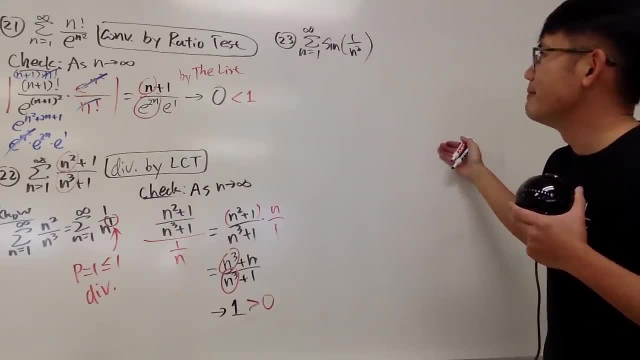 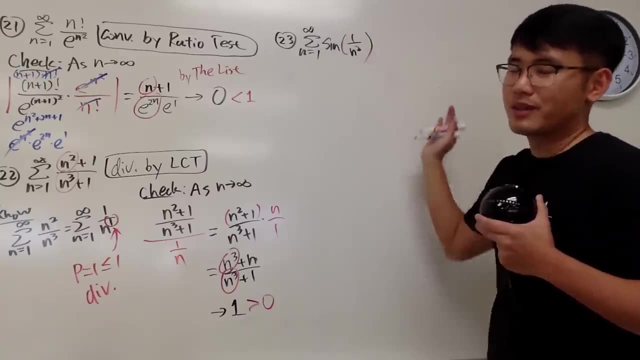 And it's decreasing. If you want, you can maybe do direct comparison test, but I'm not sure about how this is compared to less than or equal to 1 over n squared. To be honest, I don't know, And usually it's hard when you have a sine cosine, all that stuff. 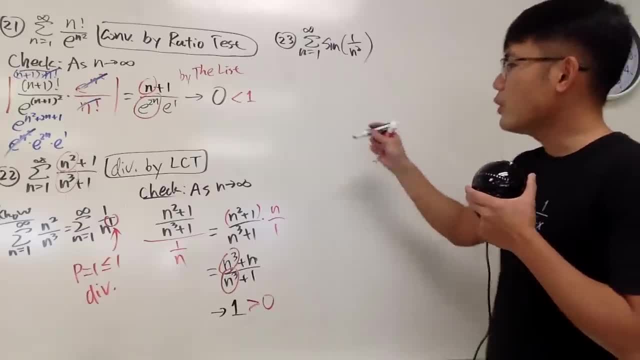 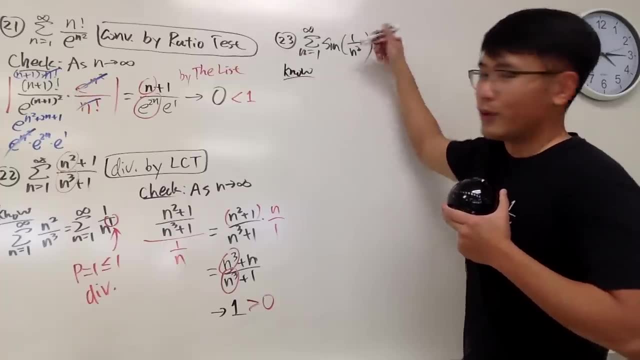 So again, let's try the limit comparison test very nicely, So I will do that right here. I have the limit comparison test in my head, Right, I'm going to use that. So this time I'll just pick the p series that we can see, which is 1 over n squared right. 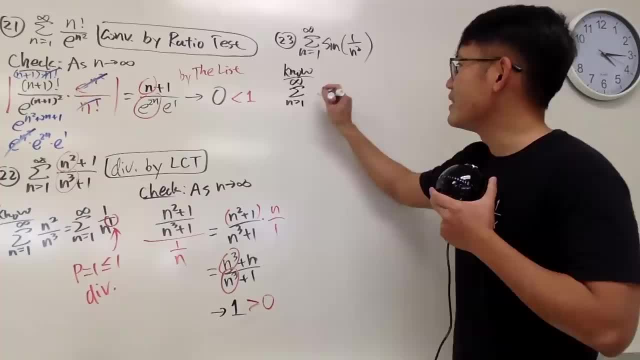 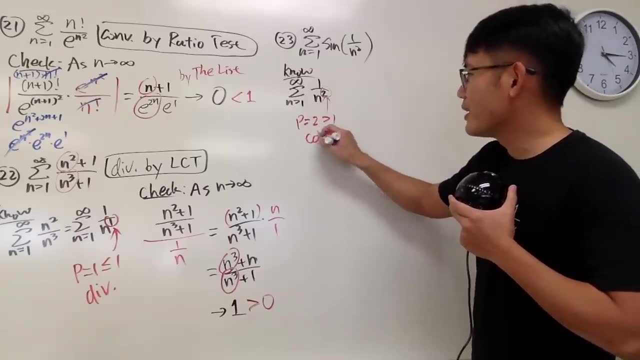 So I'll just say: we know that the sum as n goes from 1 to infinity, 1 over n squared. Here we go again. P is 2, which is greater than 1, which right here it converges right. 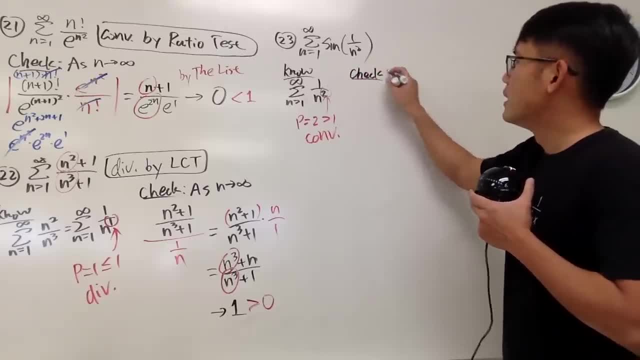 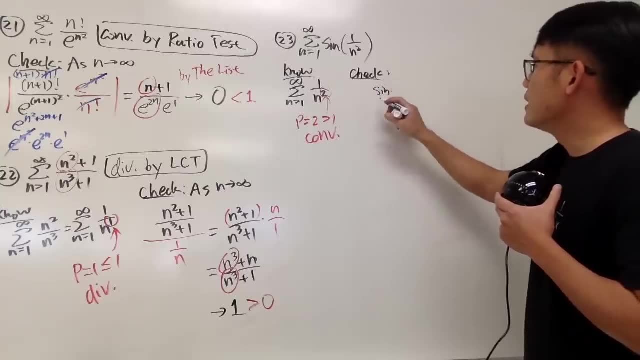 Now we are going to check. This is what we know, right? So this is what we have. So let's just put this down right here. Then we will check the sine of 1 over n, squared like this, divided by the one that we know. 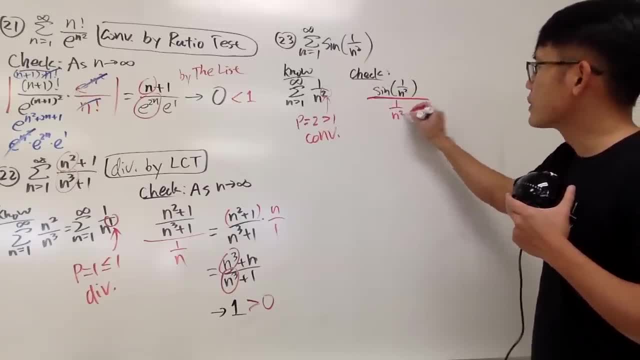 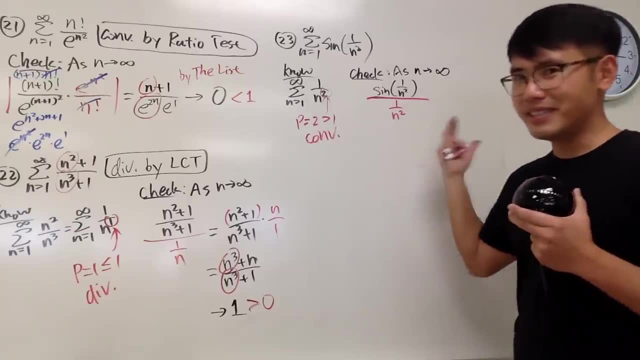 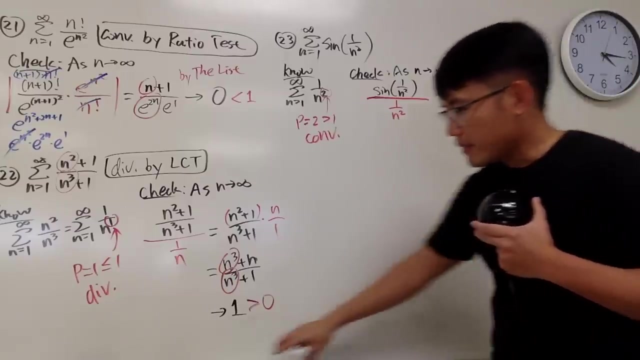 much better, which is that 1 over n, squared like this, And, of course, as n goes to infinity. And now this is just the limit again, And the beauty is that you have to make sure this and that are exactly the same, in order. 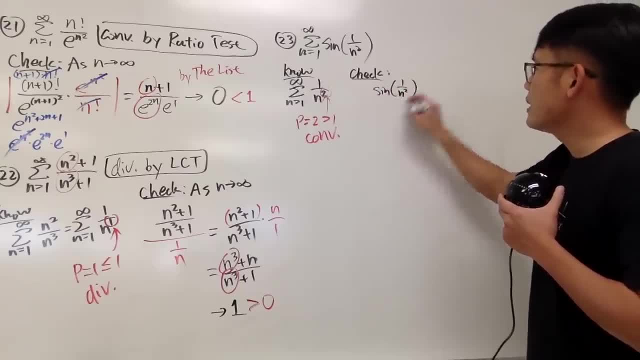 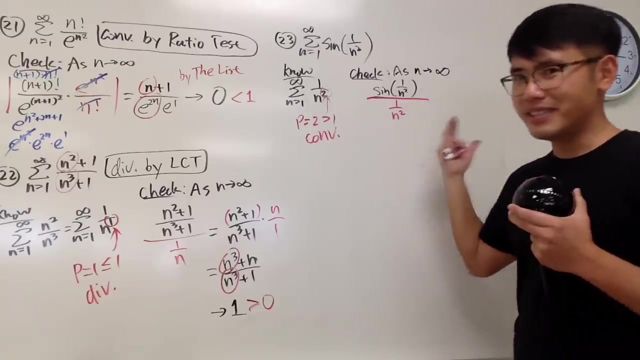 check the sine of 1 over n, squared like this, divided by the one that we know much better, which is that 1 over n squared like this, And, of course, as n goes to infinity. And now this is just the. 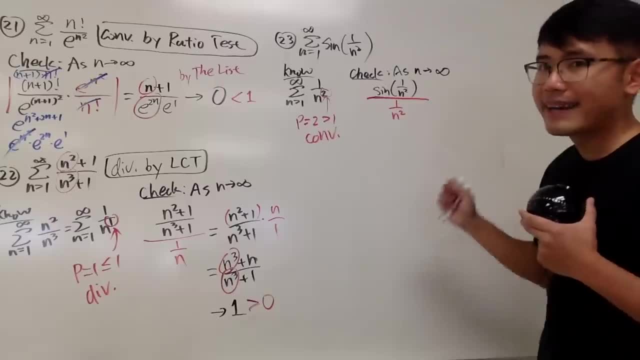 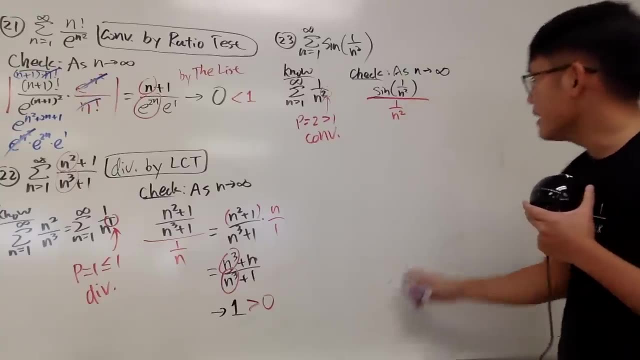 limit again, And the beauty is that you have to make sure this and that are exactly the same. Instead, in order for us to quote the limit, So you can do that, and technically they have to approach zero inside. So I will just tell. 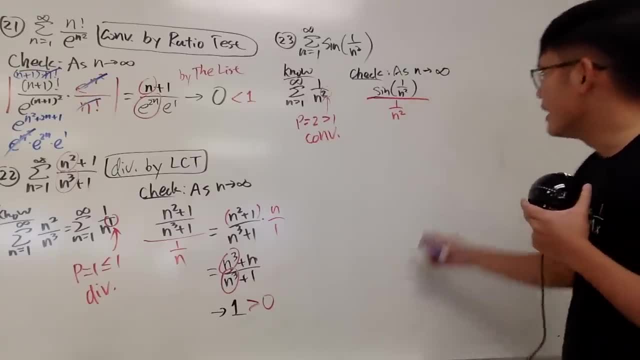 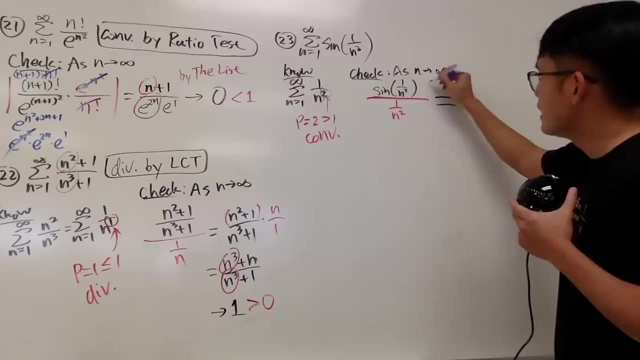 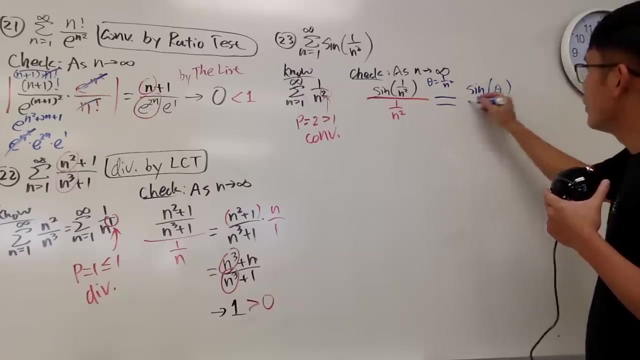 for us to quote the limit, So you can do that. And technically they have to approach 0 inside. So I will just tell you, I will just take a substitution. I will say: let theta equal 1 over n squared. So in that case I'm looking at this as sine of theta over theta, like this: 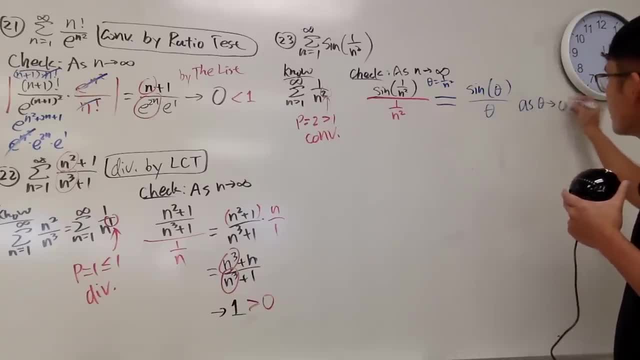 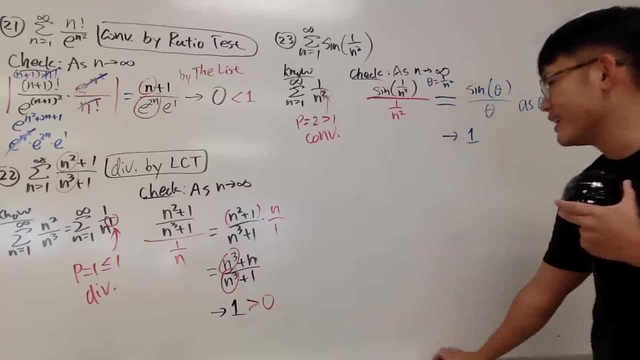 And this right here will be as theta going toward 0. You see, this right here is just equal to 1.. Very nice, Very nice. So again they are having a little bit of a problem. So again they are having a little bit of a problem. 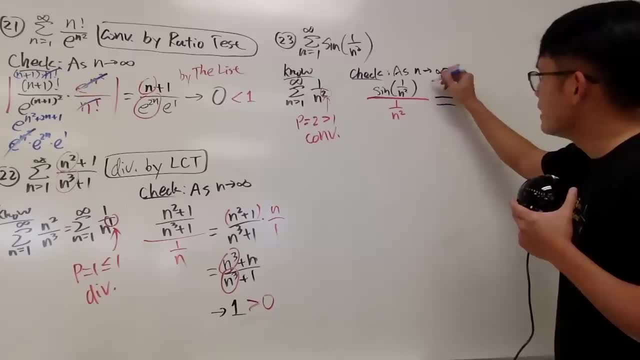 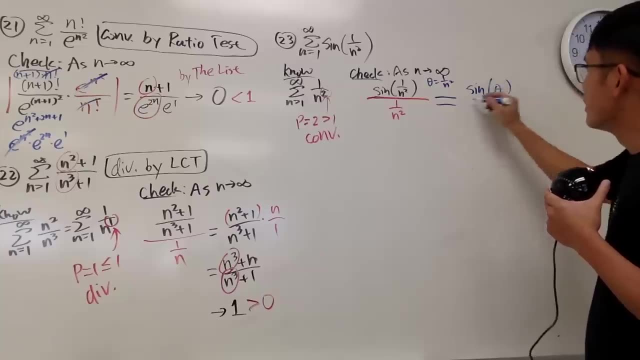 you. I will just take a substitution. I will say: let theta equal 1 over n squared. So in that case I'm looking at this as sine of theta over theta like this, And this right here will be at theta going toward zero. 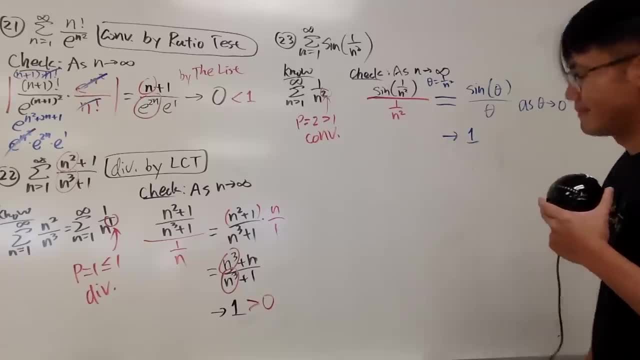 You see, this right here is just equal to 1.. Very nice, very nice. So again they are having about. they'll pretty much have the same size And of course we can utilize this. Now we can come back here and say: 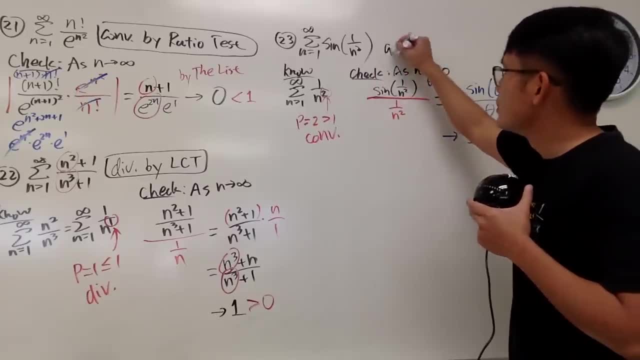 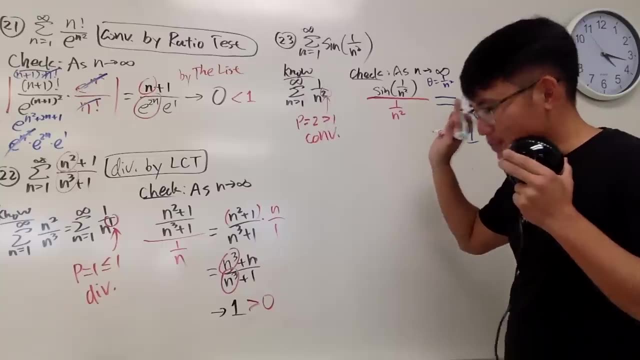 this right here also converges, Just put down also. I didn't put down also in the previous question, so I'll just put down also right here I'll just put down converges. right here I'll put down converges By the limit comparison. 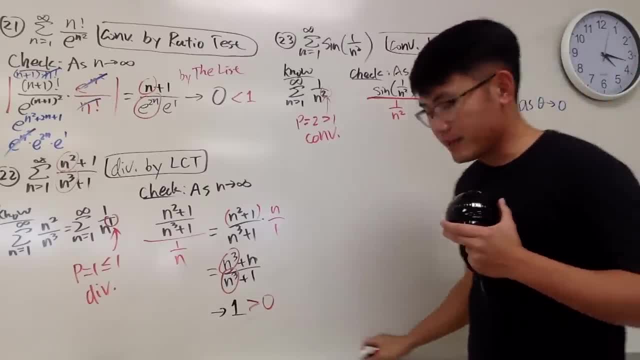 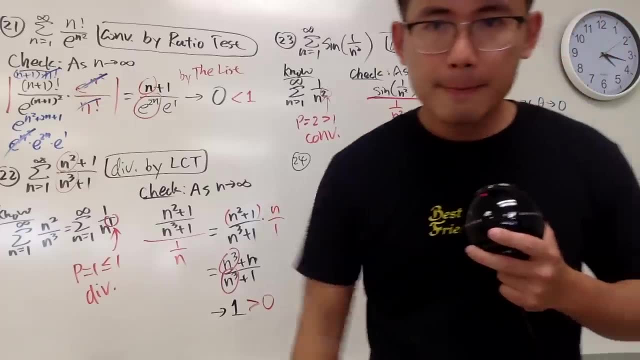 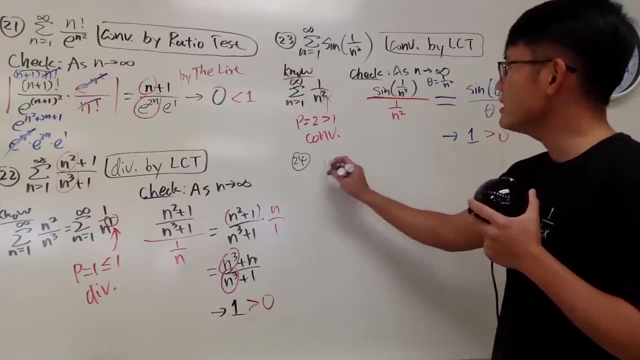 test. Phew, feel good. Now let's see number 24.. Cosine squared of 1.. Cosine, are you serious? This is the sum as n goes from 1 to infinity. cosine of 1 over n squared. 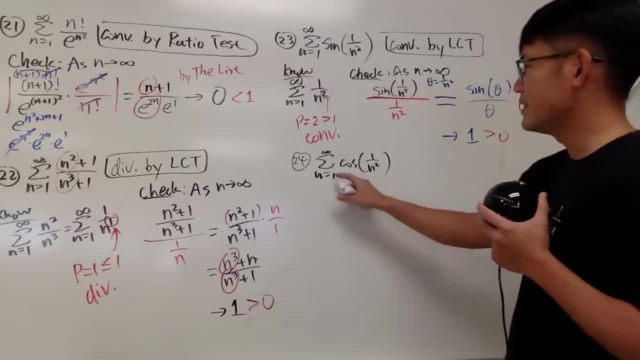 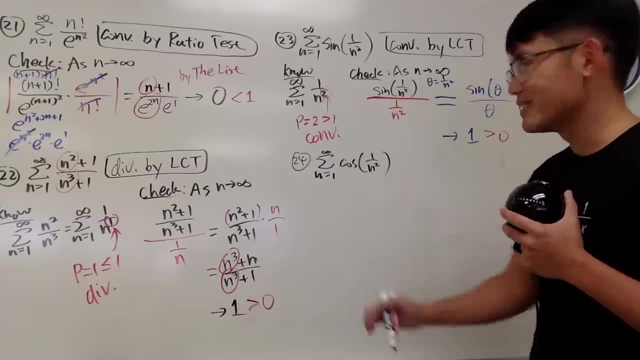 This right here is actually super easy, because if you put in infinity, in here cosine of 1 over infinity squared cosine of 0, it's just 1.. Test for divergence. So here we go. This is the check We have. 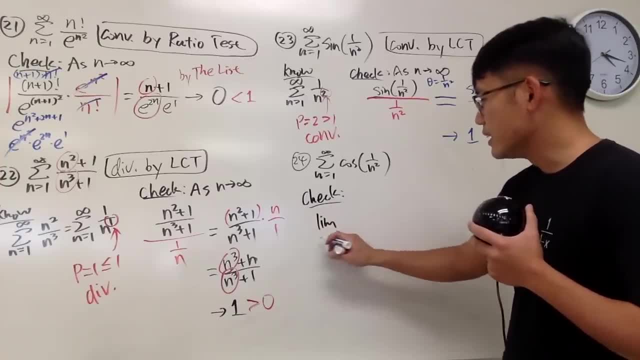 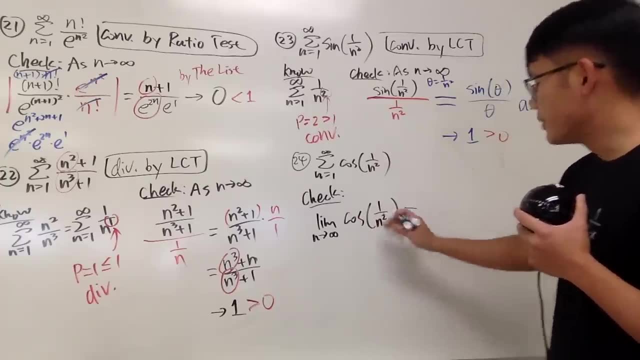 to check the test for divergence, but let me just put this down. So notice, if we take the limit as n goes to infinity of this cosine of 1 over n, squared This right here. you can put infinity inside and you can. 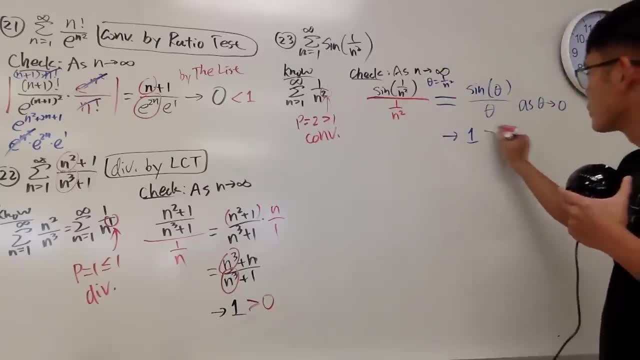 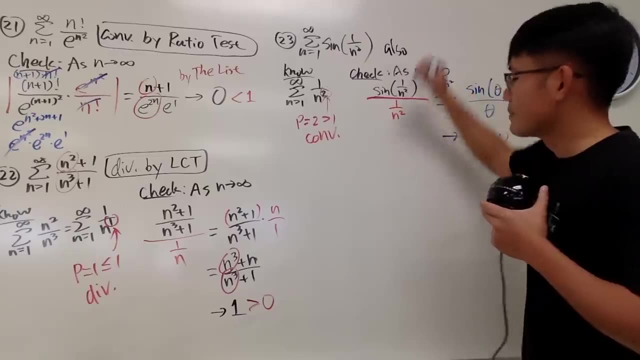 But they will pretty much have the same size And of course we can utilize this Now. we can come back here and say this: right here also converges. Just put down also. I didn't put down also in the previous question. 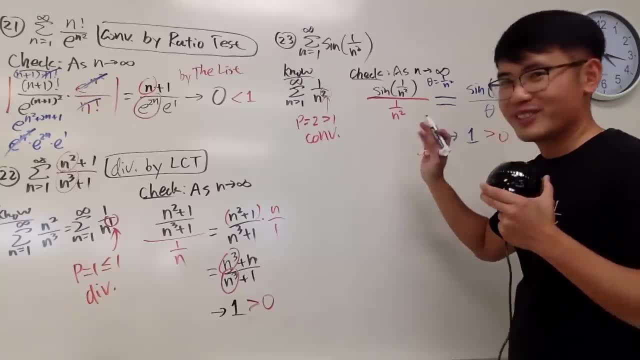 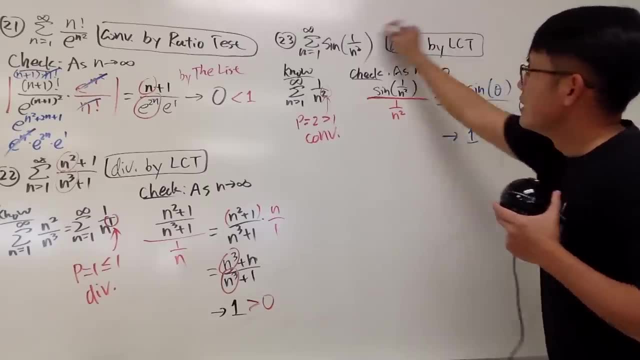 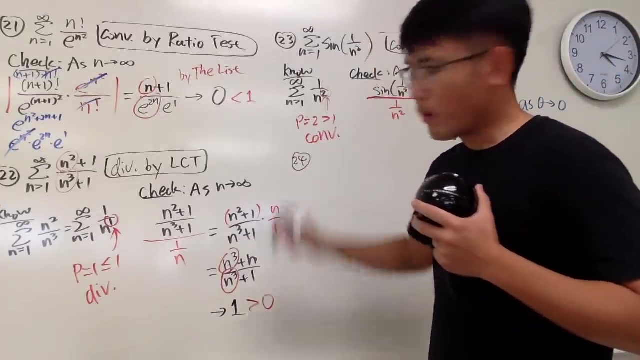 So I'll just put down. also right here I'll just put down converges. right here I'll put down converges by the limit comparison test: Feel good. Now let's see Number 24.. Cosine squared of 1.. 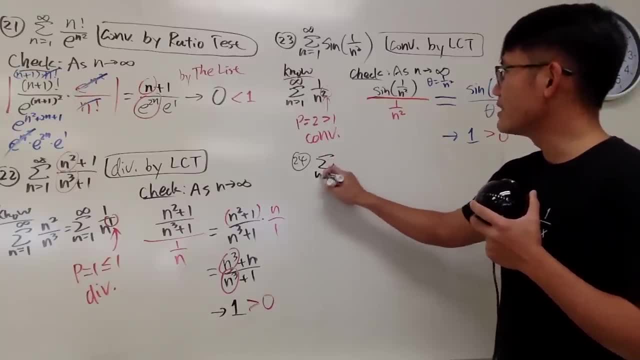 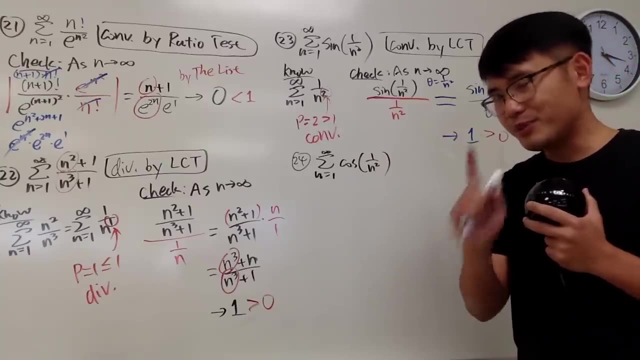 Just put the cosine, Are you serious? This is the sum as n goes from 1 to infinity. Cosine of 1 over n squared. This right here is actually super easy, Because if you put infinity in here, cosine of 1 over infinity squared. 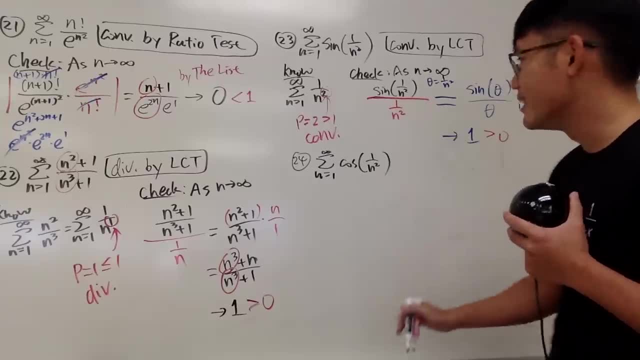 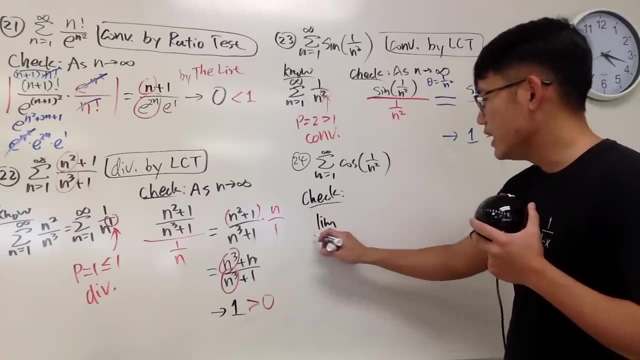 cosine of 0, it's just 1.. Test for divergence. So here we go. This is the check. We have to check the test for divergence. But let me just put this down. So notice, if you take a limit as n goes to infinity, of this cosine of 1 over n squared, 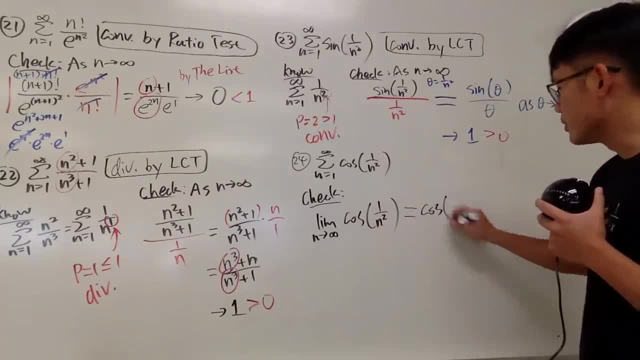 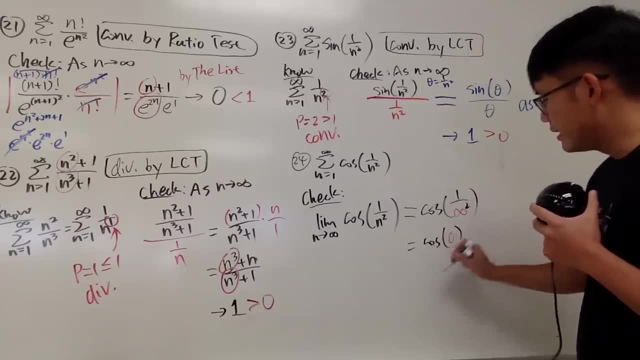 This right here: you can put infinity inside and then you can just draw a concussion along the way. So we have this right here which is just cosine of zero, And this right here is equal to 1.. And notice: if you use a test for divergence you have to indicate that 1 is not. 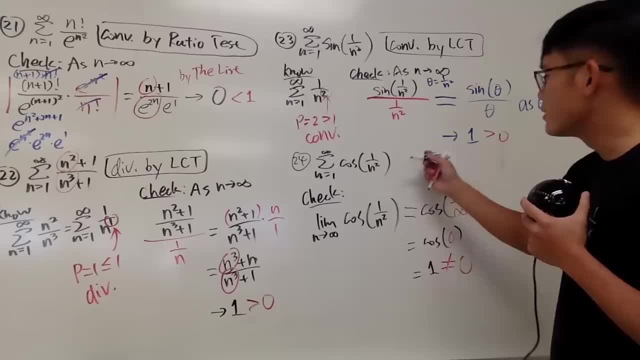 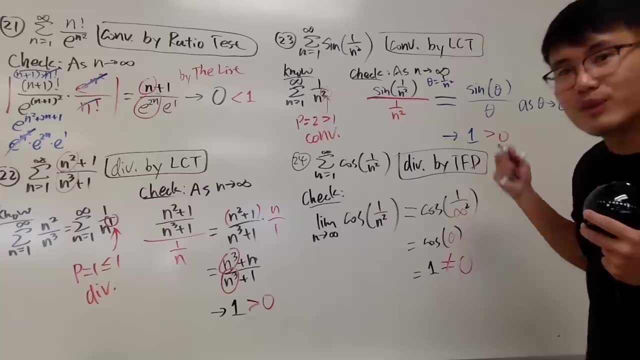 the same as zero. Therefore, you can come back here and say this right here is 0, and this right here is 0. And you can put whatever you want to do. Finally, tenth of times, it's 0.. divergence by the test for divergence like this: and with that we are done now. 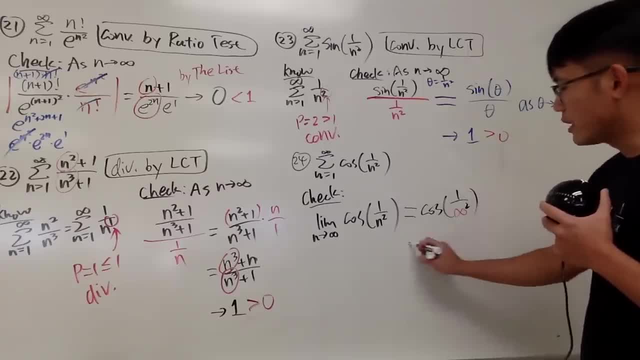 just draw a conclusion along the way. So we have this right here which is just cosine of 0, and this right here is equal to 1.. And notice, if you use the test for divergence, you have to indicate that 1 is not the same as. 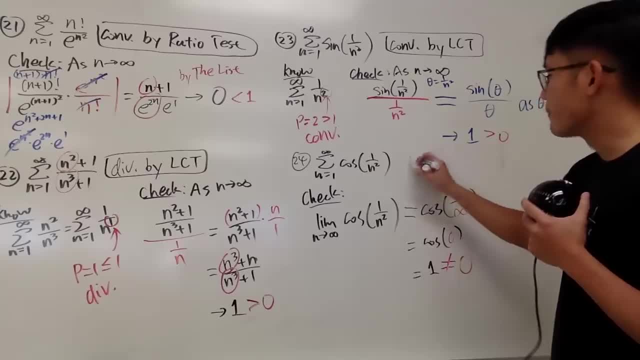 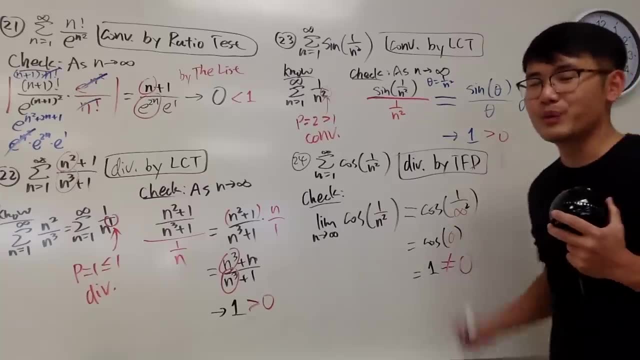 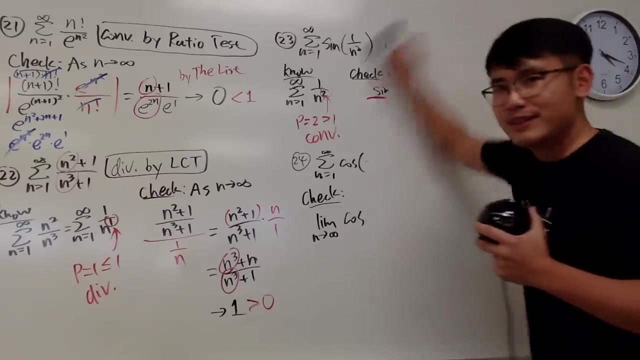 0. Therefore, you can come back here and say this right here: divergence by the test for divergence like this, And with that we are done. Now, of course, erase the board again. It's actually a lot of fun to do. 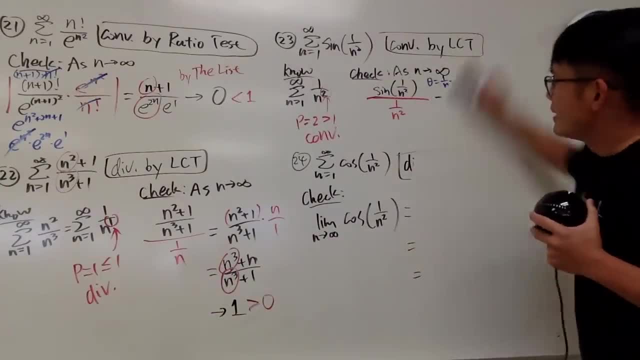 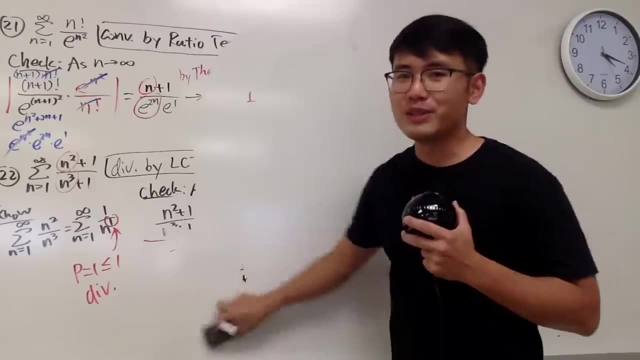 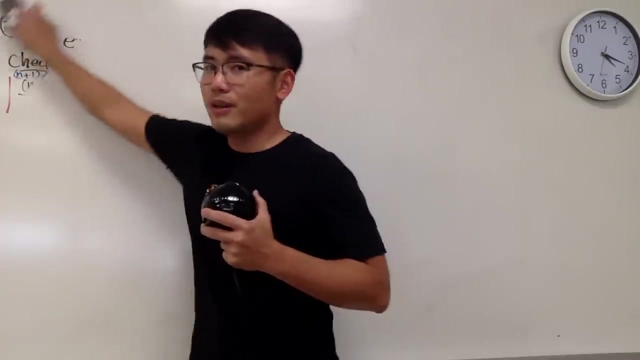 of course, erase the board again. it's actually a lot of fun to do a lot of questions at the same time for me as a teacher. I like to teach a lot of questions and in fact when I teach, I usually teach about like five hours a day or so, five, six hours, and in the past I taught longer hours and I do run. 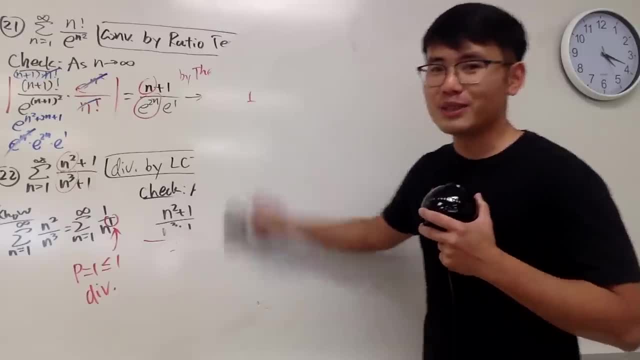 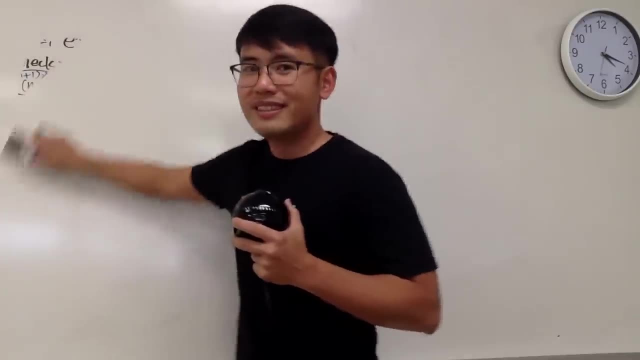 a lot of questions at the same time. For me as a teacher, I like to teach a lot of questions And in fact, when I teach, I usually teach about like 5 hours a day or so, 5-6 hours. 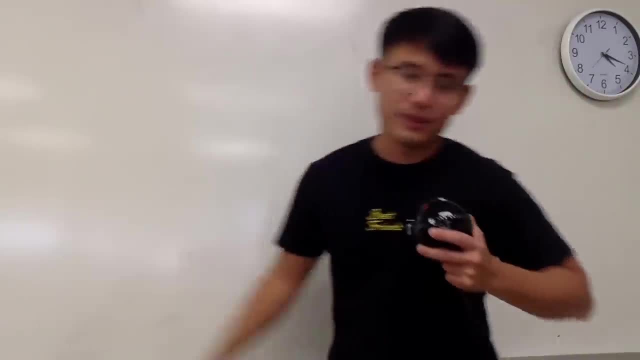 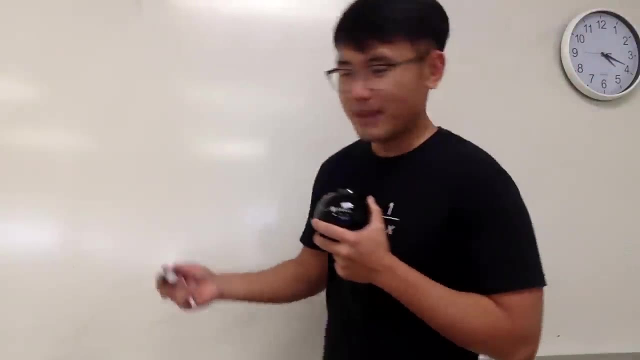 And in the past I taught longer hours And I do run marathons, so I feel good, I feel good, I feel good. Next one: we have the whole nth Coming back again. number 25, right here. 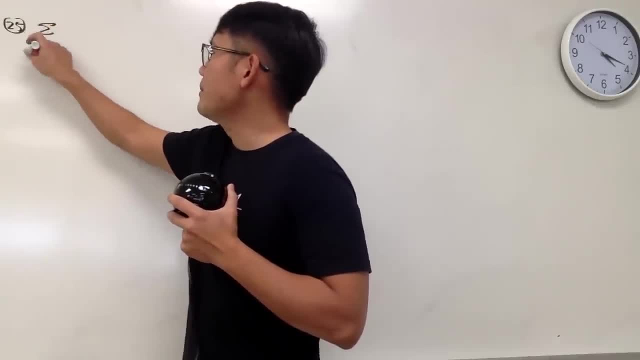 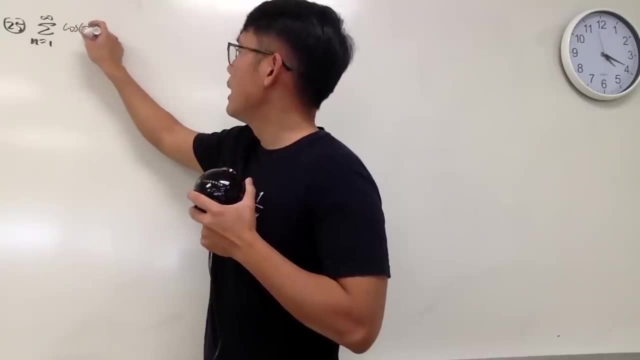 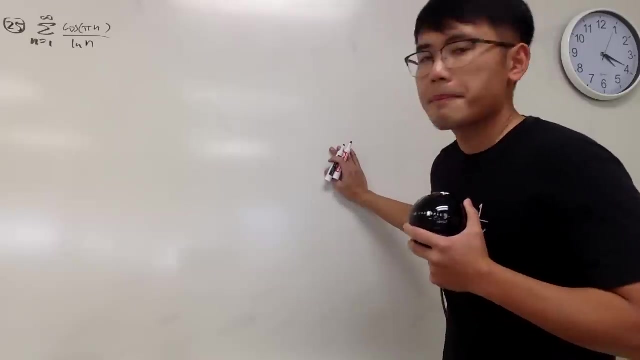 Number 25.. We have to look at the sum as n goes from 1 to infinity And we have cosine of pi n over ln, n like that. Hmm, Okay, If you want to take the absolute value. unfortunately it's bad. 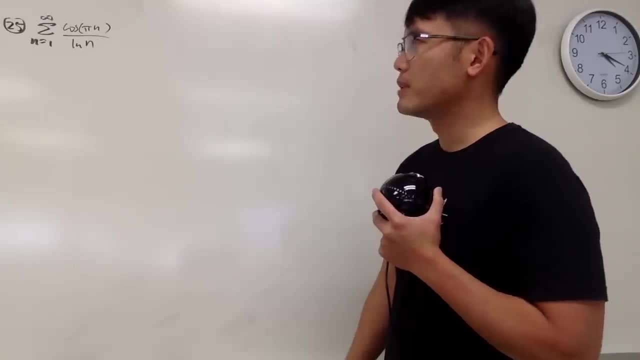 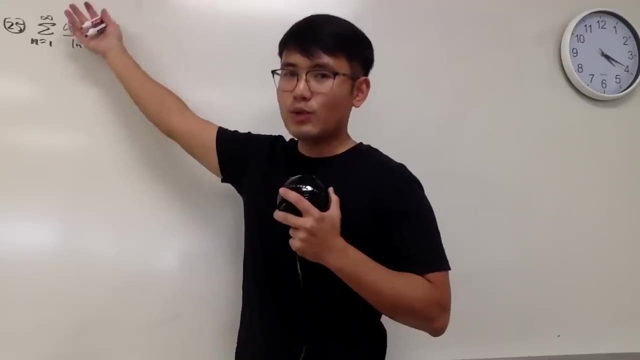 Because you end up with a divergence. Okay, If you take the absolute value, you can just replace the top with 1.. That's what I told you guys earlier. And you end up with 1 over ln n The series. for that it diverges. 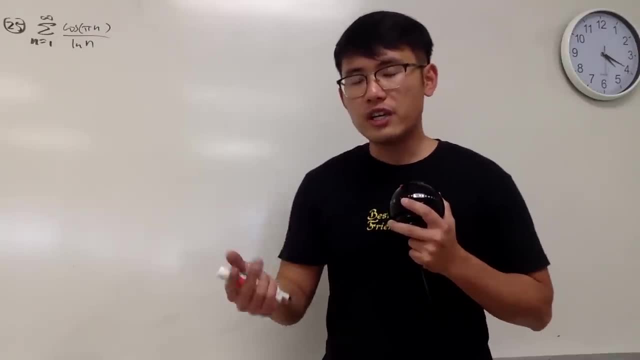 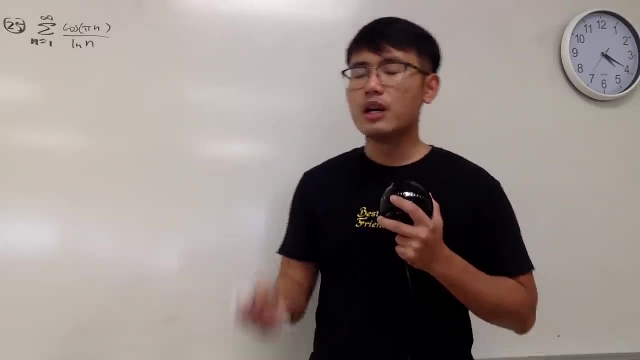 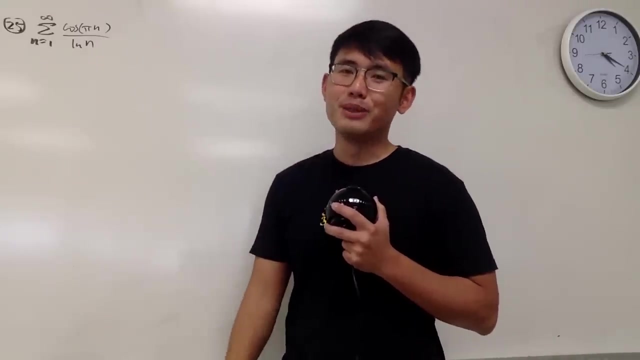 Remember, when you take the absolute value, you're trying to check for the absolute convergence And if a series converges absolutely, you can say the original series also converges, But the deal is that this series does not converge absolutely. Ah man. 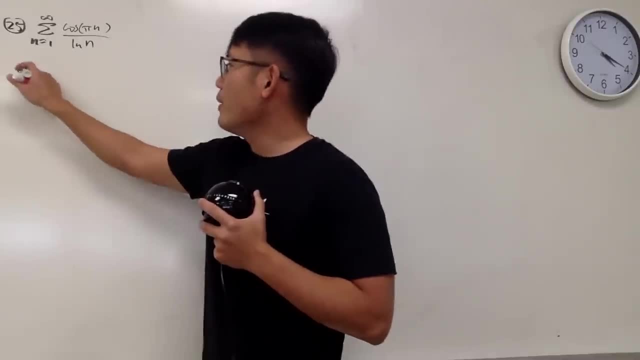 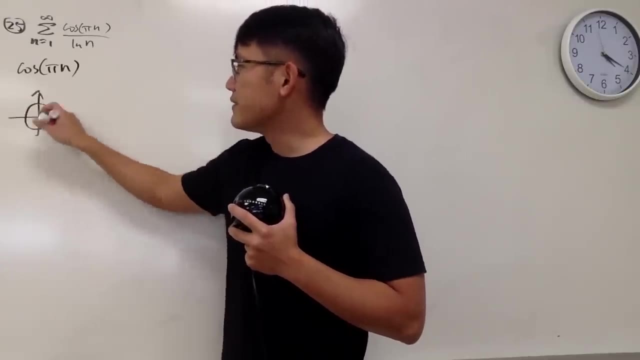 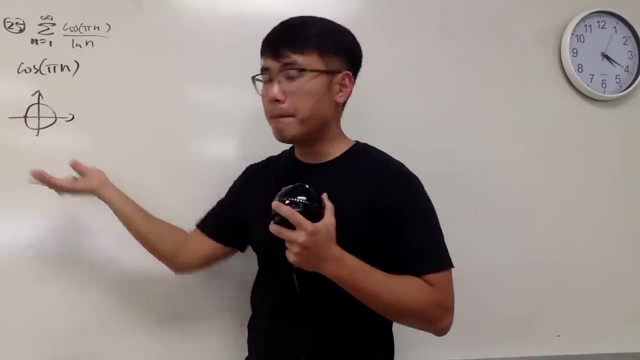 Okay, Here is the secret. Well, let's look at cosine of pi. n. Alright, Remember, cosine is the x-value on the unit circle, And when we have n equals 1 to begin with, we have cosine of pi right here, which is: 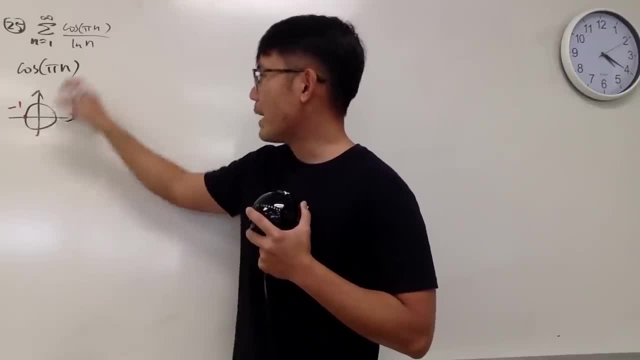 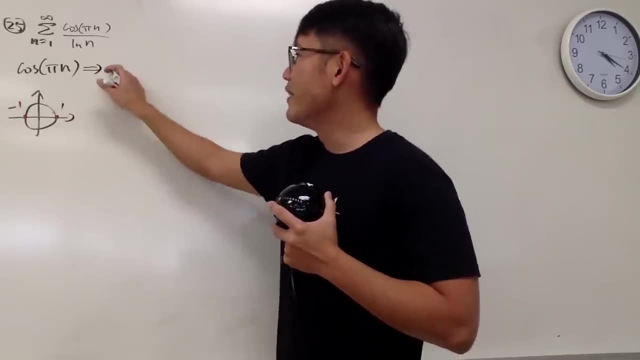 negative 1.. Right, And then cosine of 2 pi is going to be 1.. And then negative 1, and so on. So this right here is secretly producing negative 1, 1, negative 1, 1, negative 1, 1, and so on. 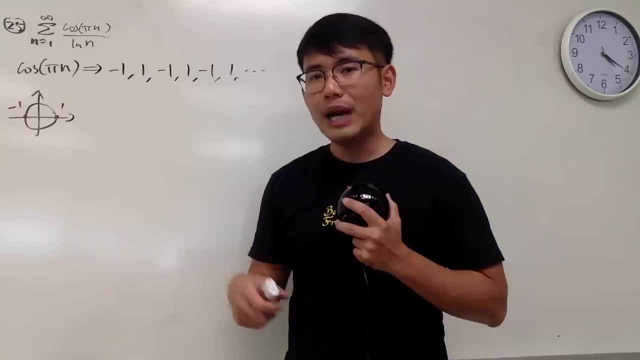 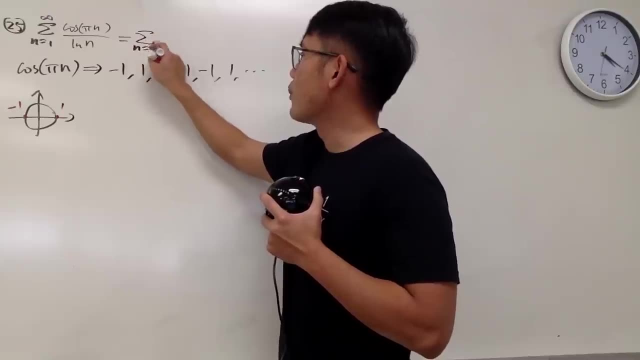 In other words, this is actually just an alternating series, So we have to do the usual test with the bn thing, Right? So notice this right here is actually the same as the sum, as n goes from 1 to infinity. And again for all these things, right? 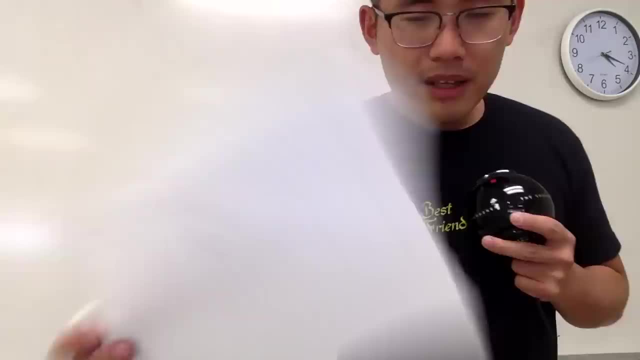 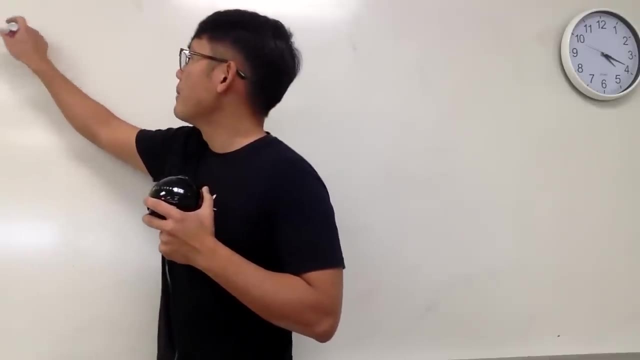 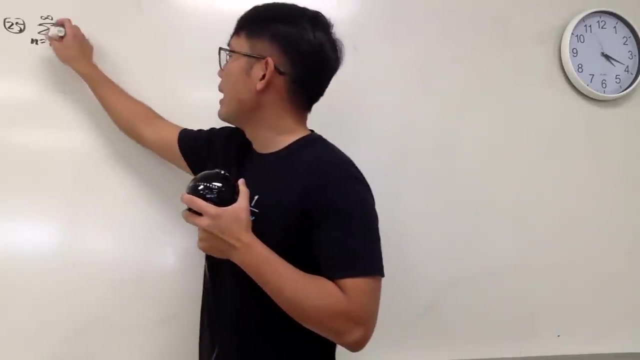 marathons. so I feel good, I feel good, I feel good. next one: we have the hell and coming back again, number 25. right here, number 25, we have to look at the sum as n goes from 1 to infinity and we have cosine of pi n over lnn, like. 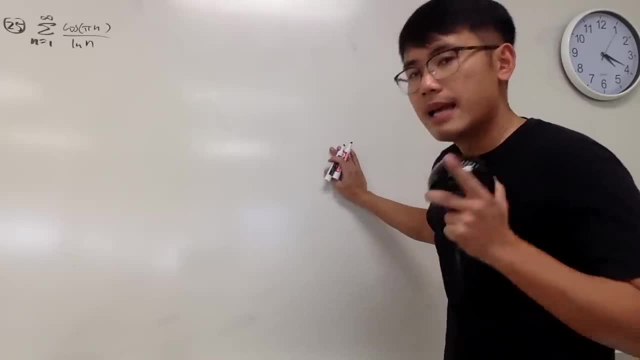 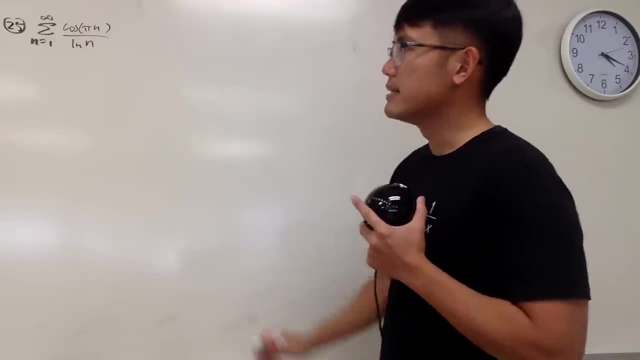 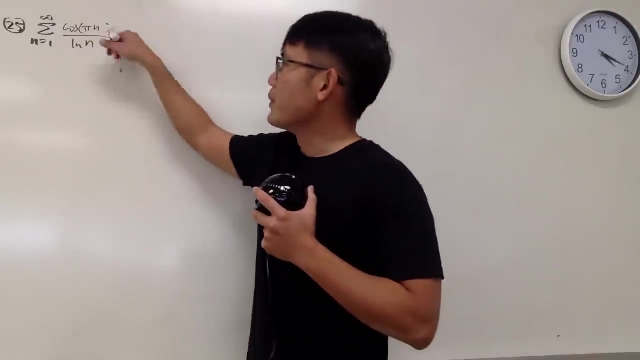 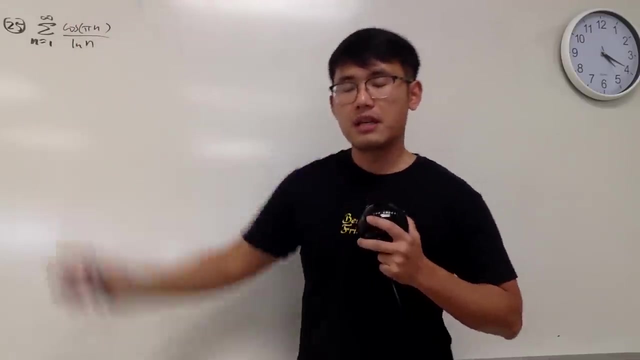 you that, hmm, okay, if you want to take the absolute value- fortunately it's bad because you end out with a divergent- okay, if you take the absolute value, you can just replace the top with 1- that's why I told you guys earlier- and you end out with 1 over lnn the series. for that it diverges, remember? 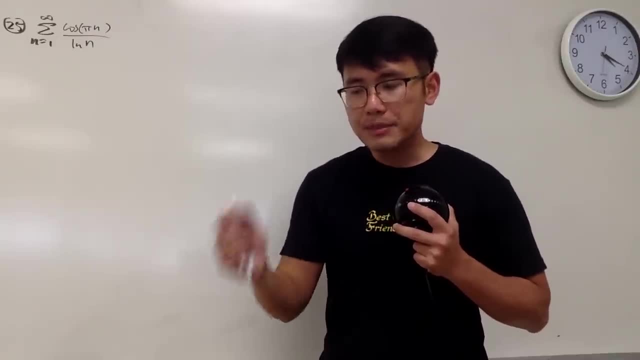 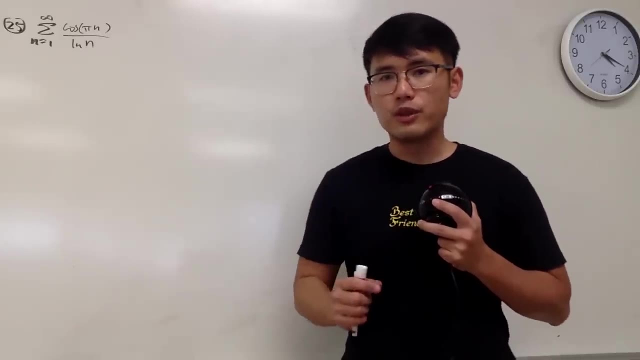 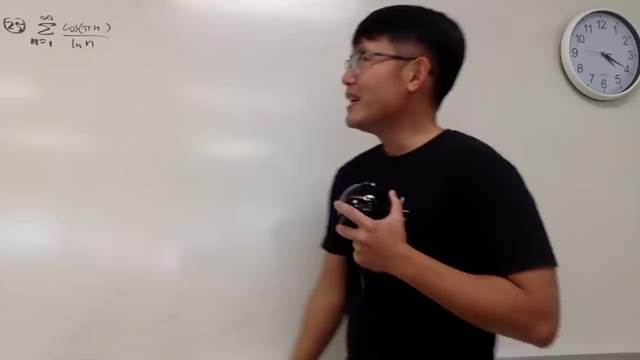 when you take the absolute value, you're trying to check for the absolute component, convergence, and if a series it converges absolutely, you can say the original series also converges, but the deal is that this series does not converge absolutely. ah man, okay, here is the secret. well, let's look at cosine of pi. 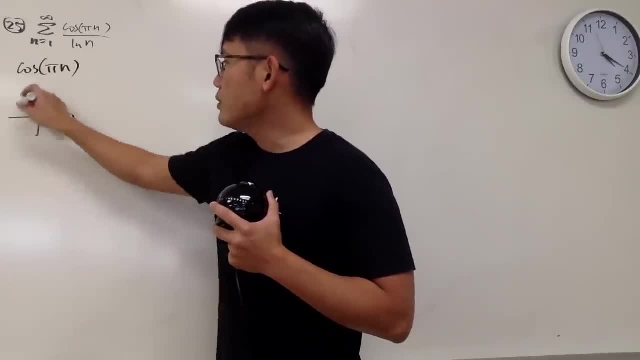 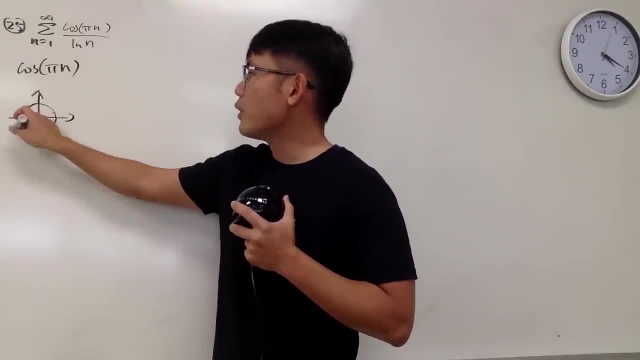 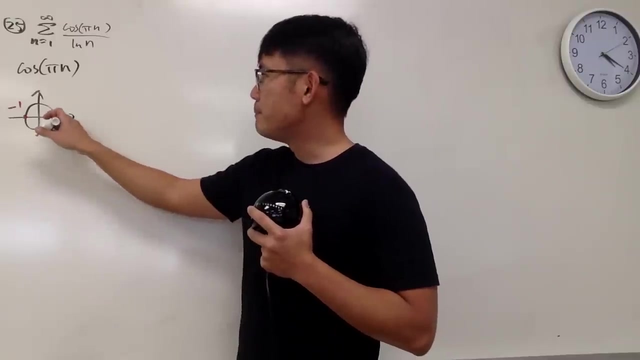 n right. remember, cosine is the X value on the unit circle and when we have n equals 1 to begin with, and when we have n equals 1 to begin with, we have cosine of pi right here, which is negative 1 right, and then cosine of 2 pi. 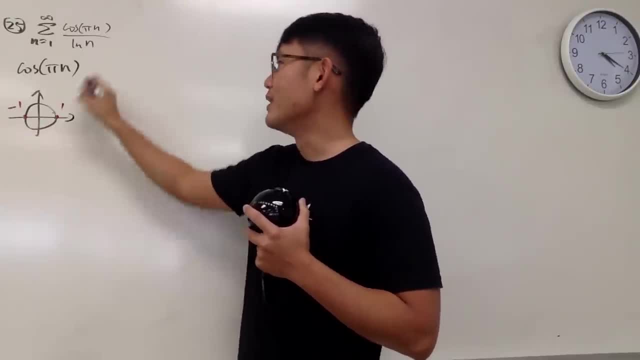 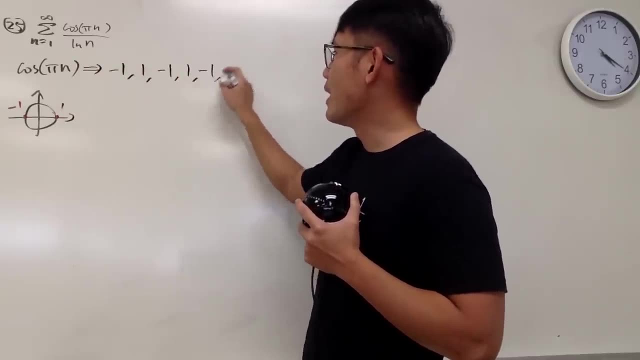 is going to be 1, and then negative 1, so on. so this right here is secretly producing negative 1, 1, negative 1, 1, negative 1, 1 and so on. in another word, this is actually just an alternating series, so we have to just do the usual. 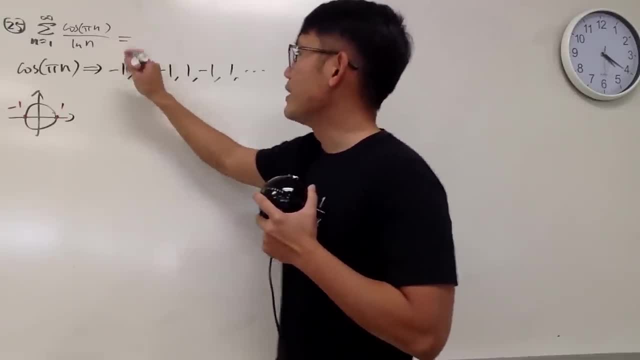 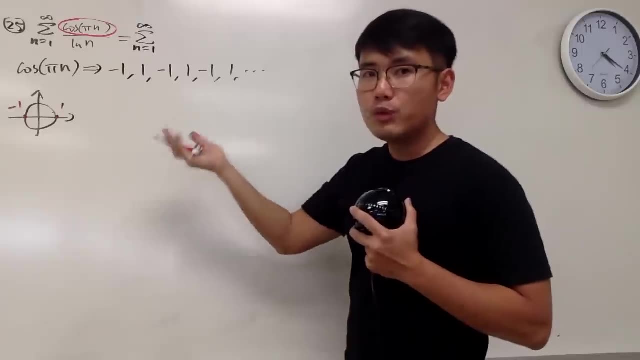 test with the b-n thing right. so notice this right here is actually the same as the sum, as n goes from 1 to infinity and again for all these things right here we can rewrite this as negative 1, and because the first term is negative 1, so I just put. 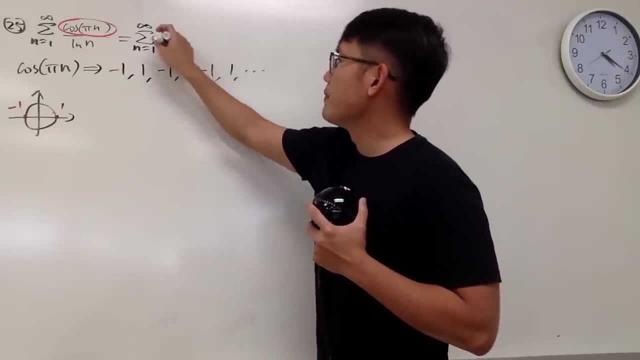 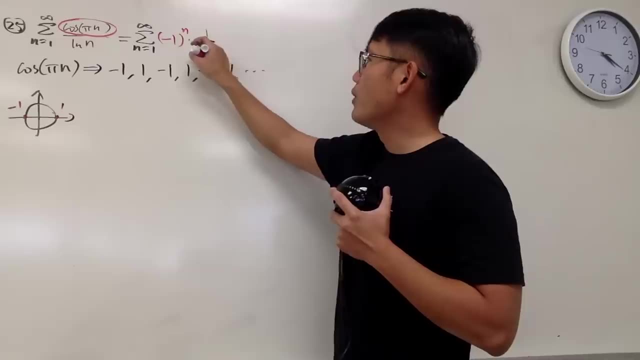 here we can rewrite this as negative 1.. And because the first term is negative 1, so I just put this down as to the nth power, And then we multiply by 1 over natural log of n And we will take this guy right. 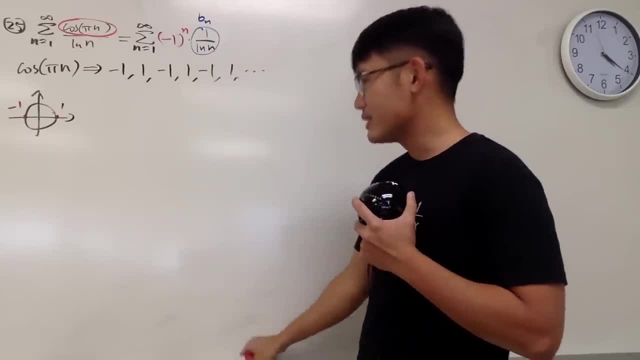 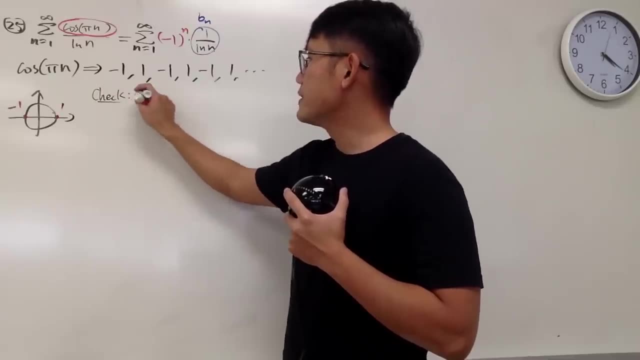 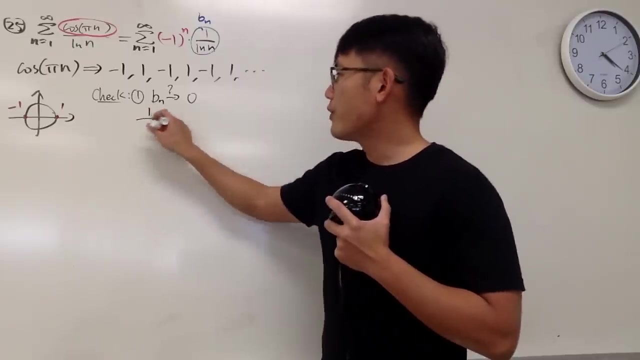 here to be our bn And of course, let's do the usual check Right here. let's go ahead and say we are going to check first thing: does bn go to 0 as n goes to infinity? Well, 1 over ln. 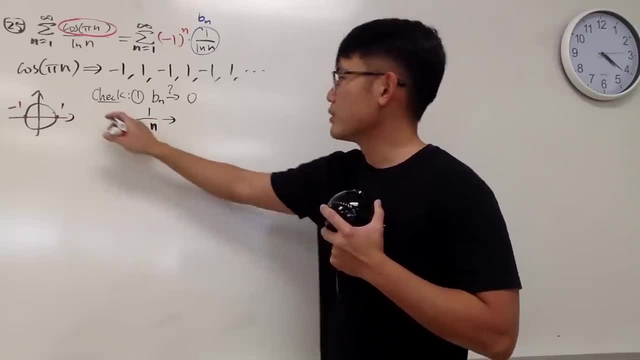 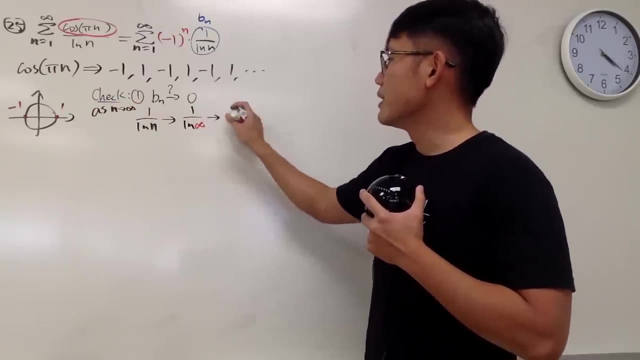 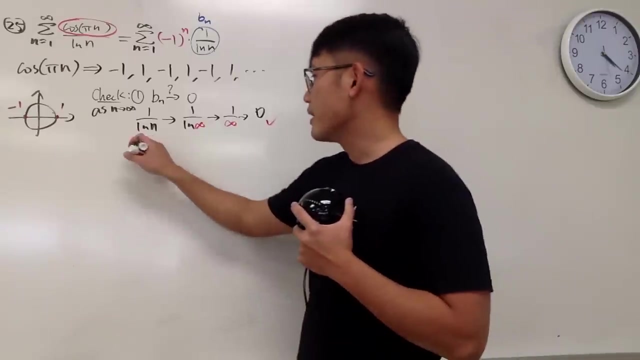 n does go to infinity. I'll just put down somewhere: as n goes to infinity, This is 1 over ln infinity. Of course, that's 1 over infinity. that goes to 0.. So the first thing, check. Second thing: 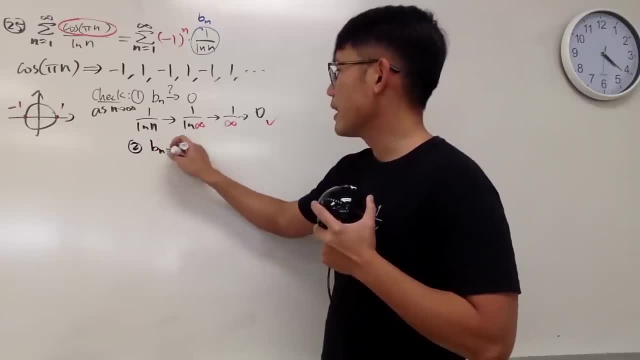 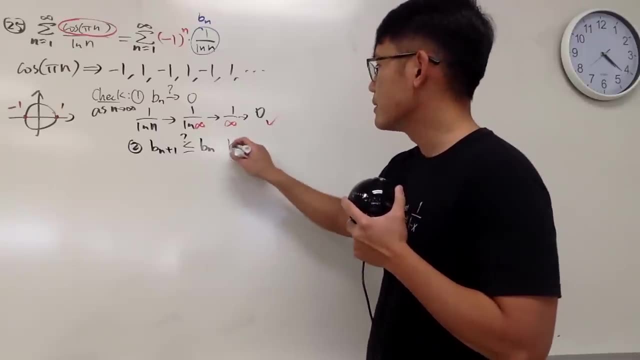 does bn decrease, bn plus 1? is this less than or equal to bn? right here, as n is bigger than or equal to 1.. Right, I'll just put this down, For n is bigger than or equal to 1.. 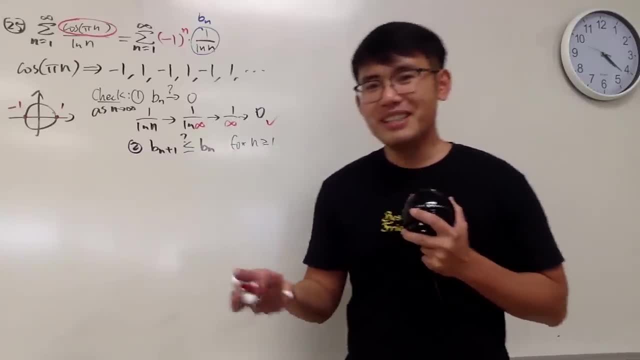 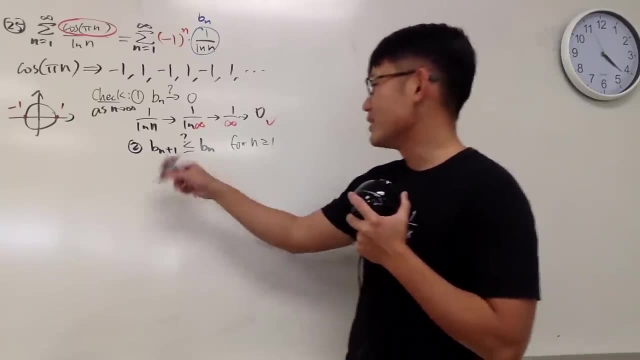 Well, the truth is that log is an increasing function, so when you divide it becomes a decreasing function. so that's a beauty, But let's show work right here. real quick. This is 1 over ln of n plus 1.. 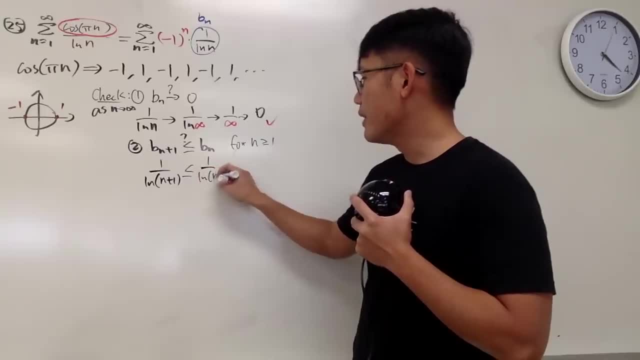 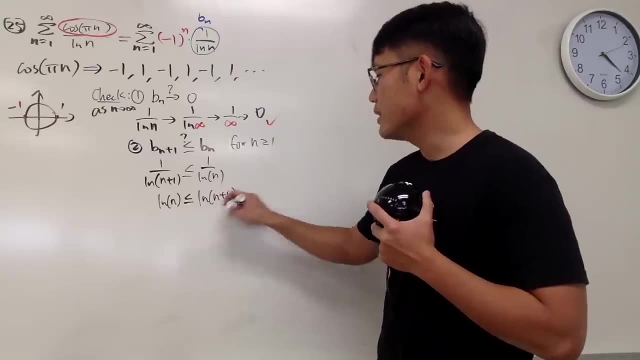 And this right here is less than or equal to 1 over ln n like this. And if you would like, you can just cross multiply as ln n less than or equal to ln of n plus 1.. And if you really want, you can just do e to this: 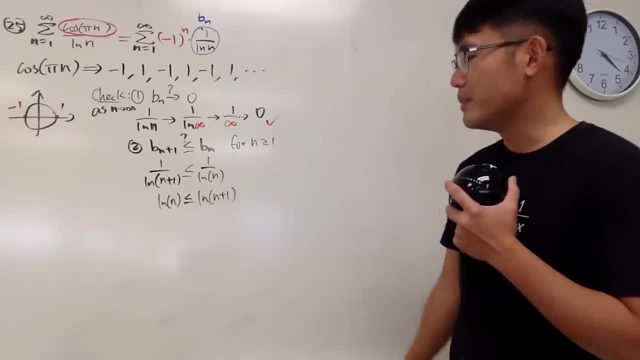 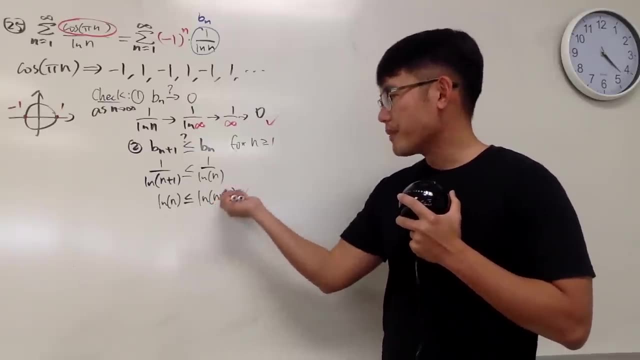 power, e to that power, and e is also an increasing function over there, so you don't have to flip the inequality sign. Anyway, this right here is true. right. Increasing function means if the bigger the inside, the bigger the outside, the output. 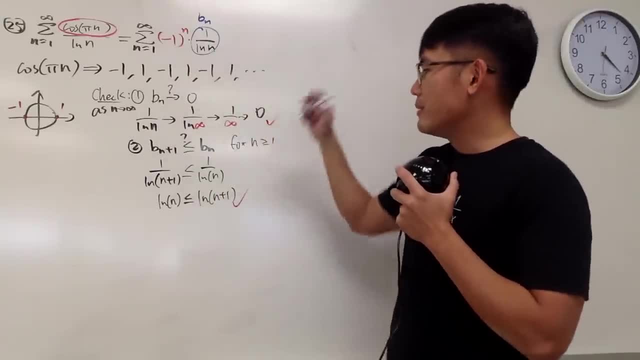 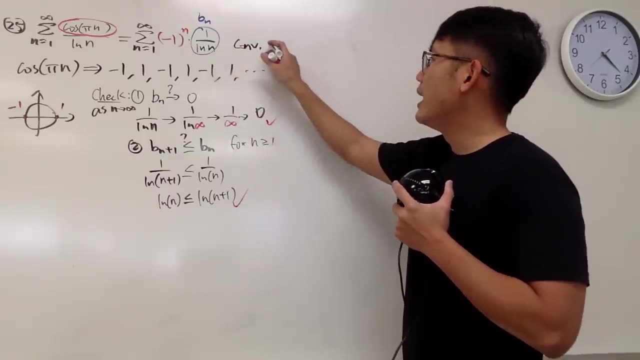 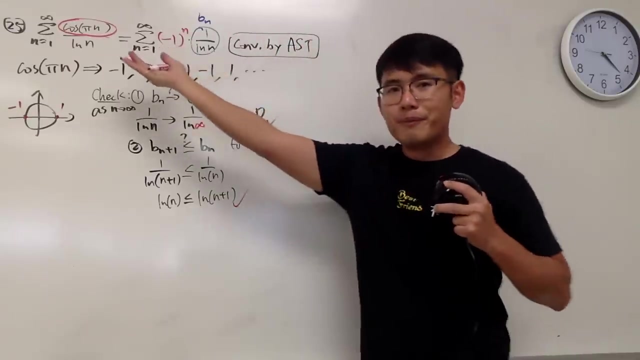 So this right here is also true. So, anyway, this right here, both of them are true, right. So we can move on and draw a conclusion that this right here does converge, and it converges because the alternating series test Right. So 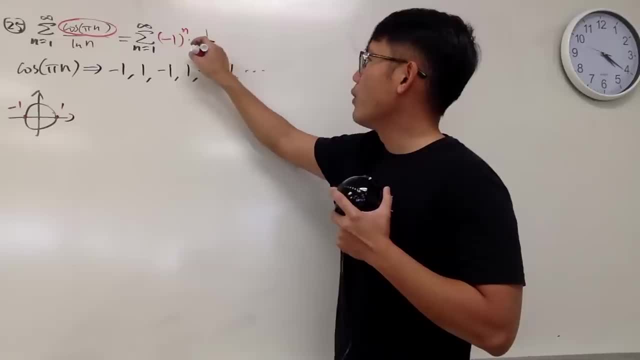 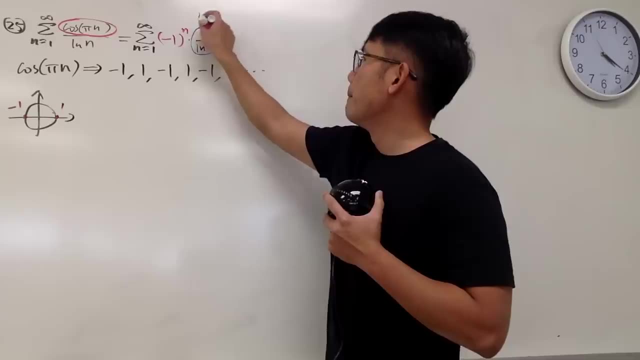 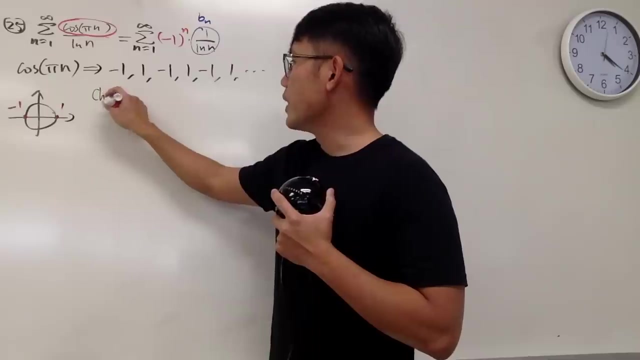 this down as to the nth power and then we multiply by 1 over natural log of n and we will take this guy right here to be our vn and of course let's do the usual check Right here. let's go ahead and say we are going to check First thing: does bn go to 0 as? 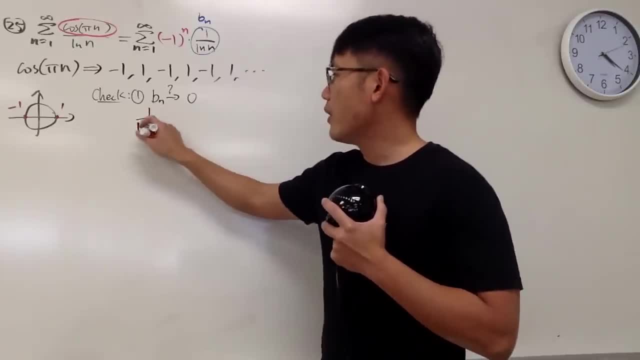 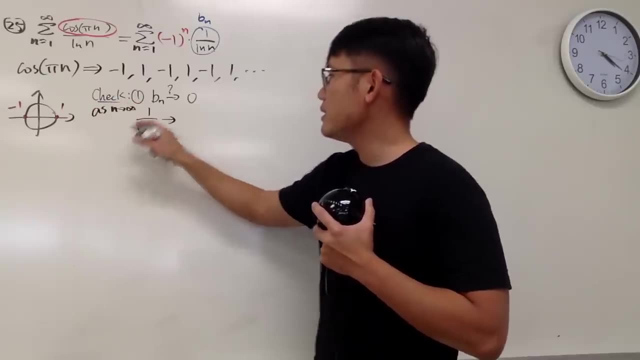 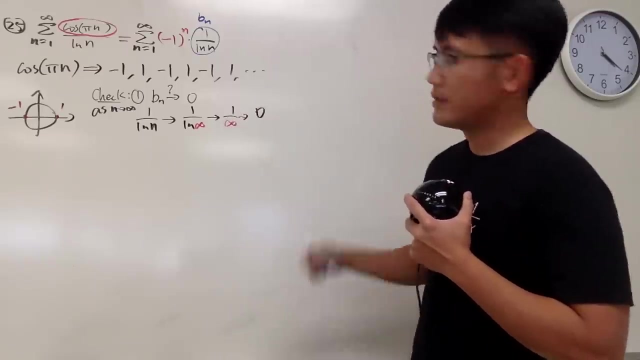 n goes to infinity. Well, 1 over ln n does go to infinity. I'll just put down somewhere: as n goes to infinity, this is 1 over ln infinity. of course that's 1 over infinity that goes to 0.. So the first thing checks. 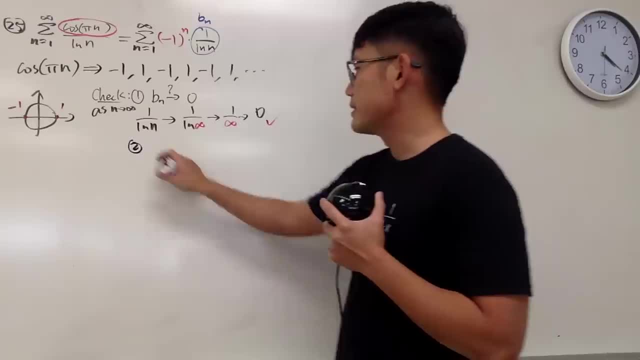 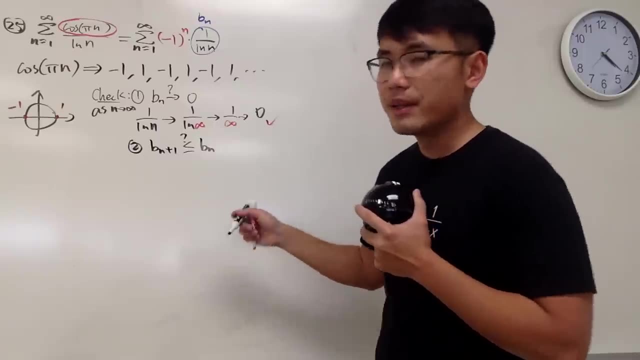 Second thing: let's go ahead and say we are going to check. First thing: does bn go to infinity? Again, does bn decrease, bn plus 1, is this less than or equal to bn? right, here, as n is bigger than or equal to 1, right, Let's just put this down, For n is bigger. 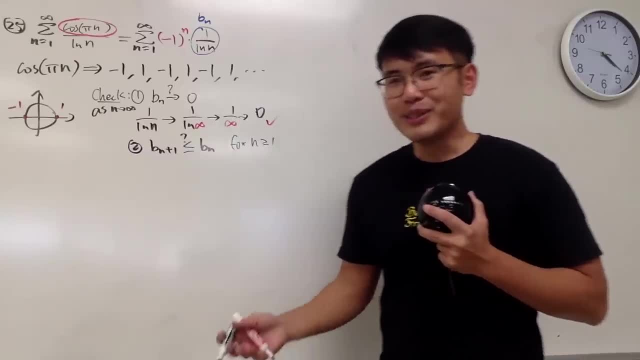 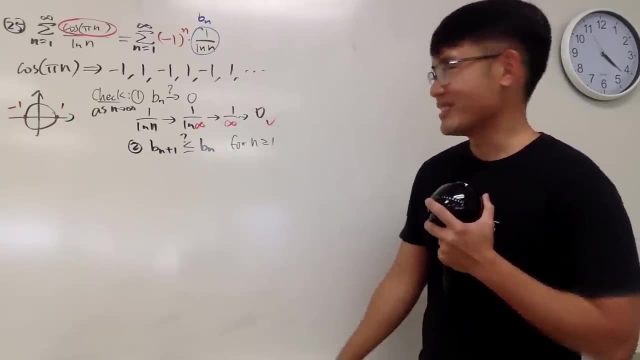 than or equal to 1.. Well, the truth is that log is an increasing function, so when you divide it becomes a decreasing function. so that's a beauty, but let's show work right here. real quick, This is 1 over ln n. 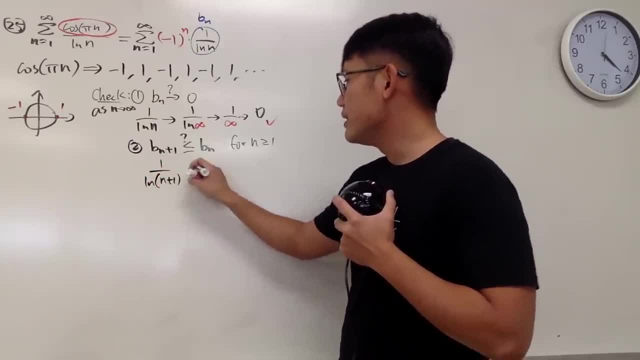 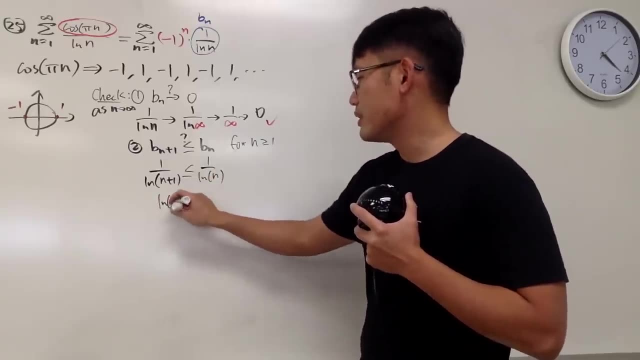 So I can see that this is just a decreasing function. so I can just say: well, bn. if I multiply this it's going to be a decreasing function, right? So I can just say: bn plus 1, right here is equal to 1 over ln n, And this right here is less than or equal to 1. 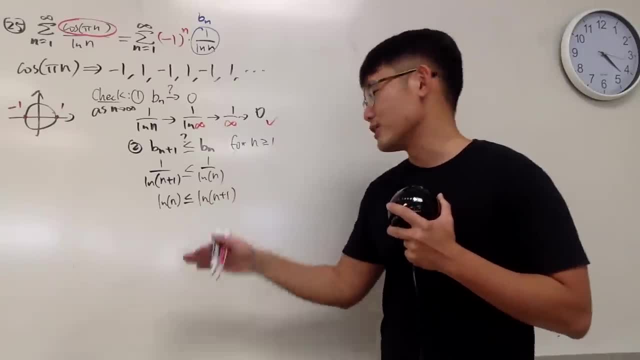 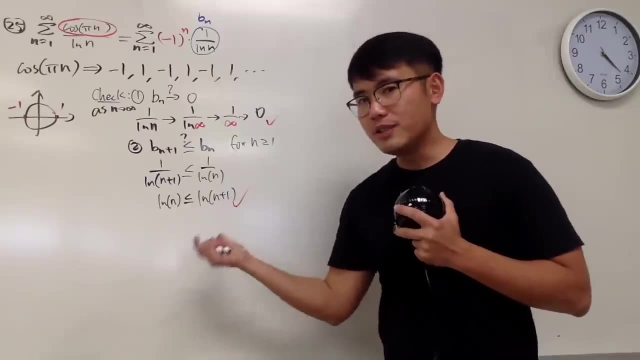 over ln n like this, And if you would like, you can just cross multiply this ln n less than or equal to ln of n plus 1.. And if you really want, you can just do e to this power, e to that power, and e is also an increasing function over there, so you don't have to flip. 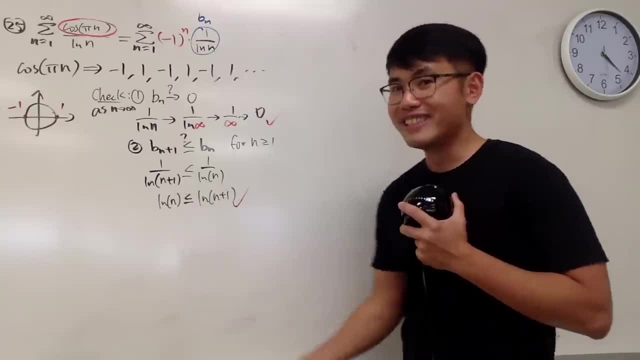 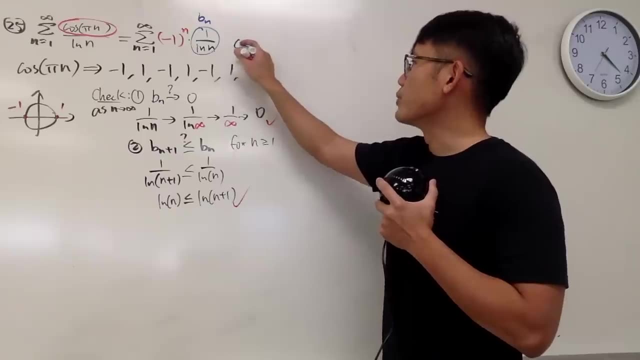 the inequality side. Anyway, this right here is true right. Increasing function means if the bigger the inside the, the bigger the outside the output. so this right here is also true. so anyway, this right here, both of them are true right. so we can move on to a conclusion that this right here does converge. 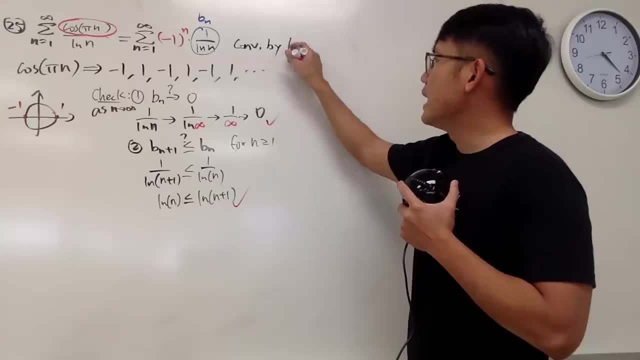 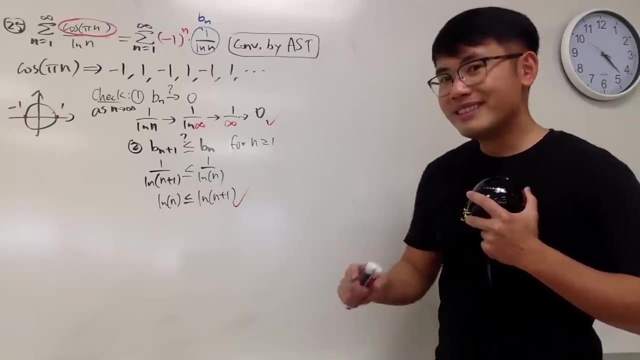 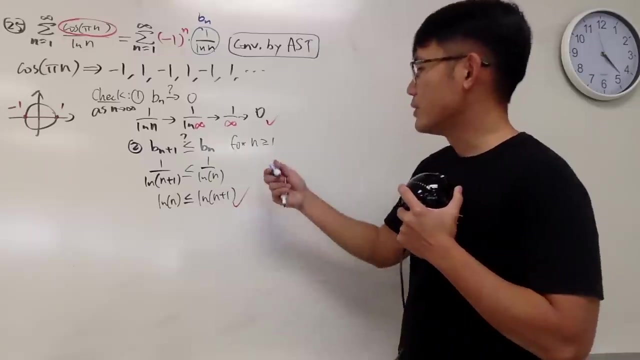 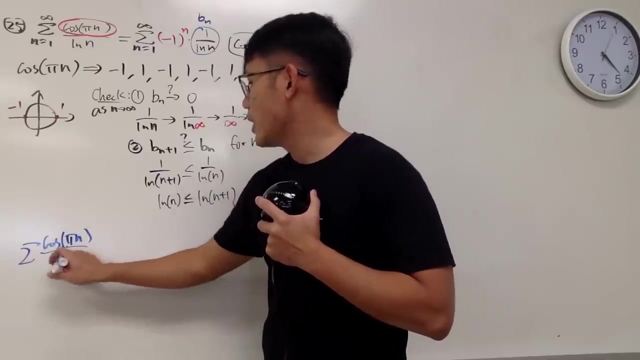 and it converges because the alternating series test right. so um, cosine of pi, n. and again, if you take the absence value, unfortunately this right here does not converge absolutely. so i will just tell you: uh, this, right here, the sum as cosine of pi, n, l and n, right here is conditional convergence. 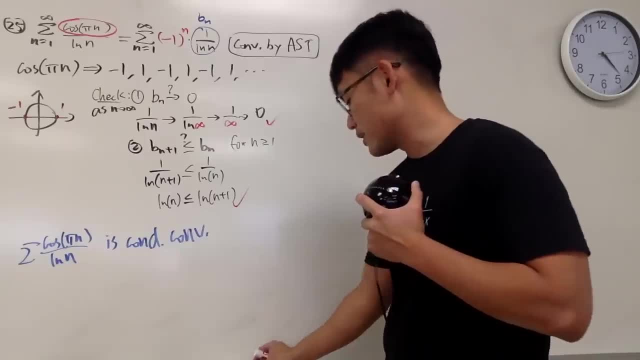 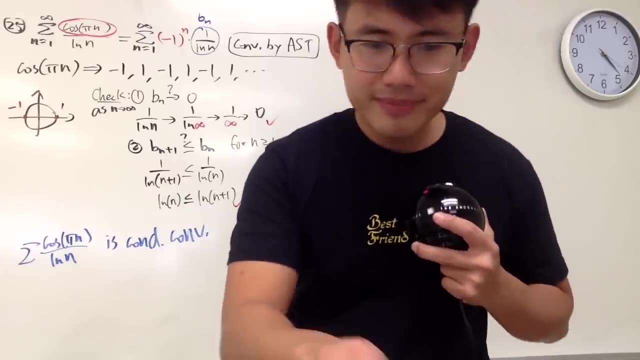 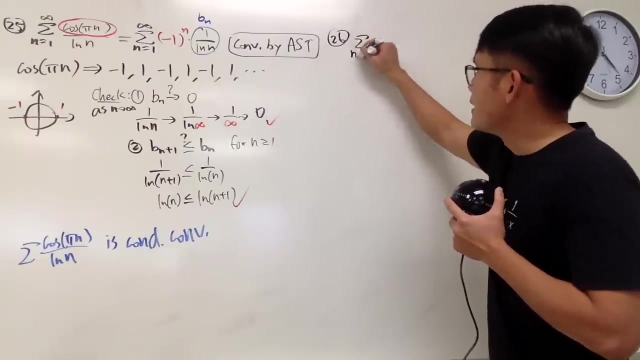 right, because if you take the absolute value, it does not work, it does not converge. okay, so that's the idea. now, moving on to hopefully another easy one, number 26, right, 26. here we have the sum, as n goes from 1 to infinity, and we are going to have 2n plus 1 to the nth power. 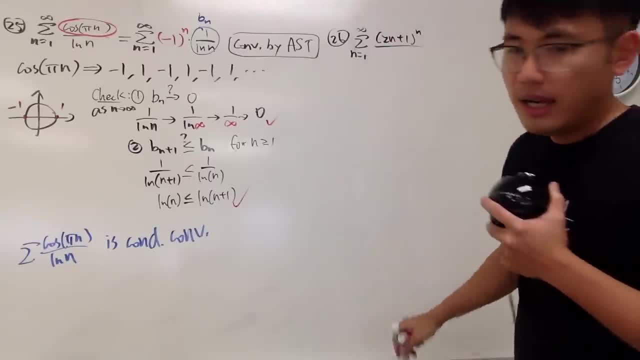 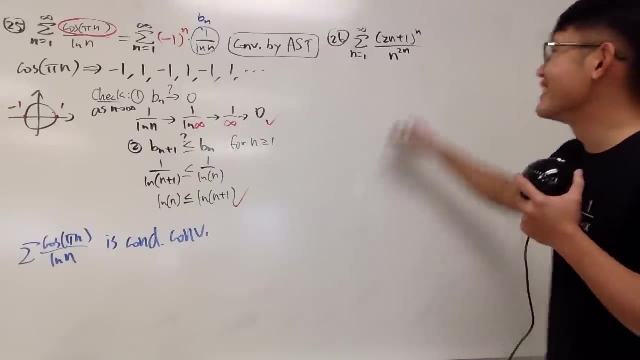 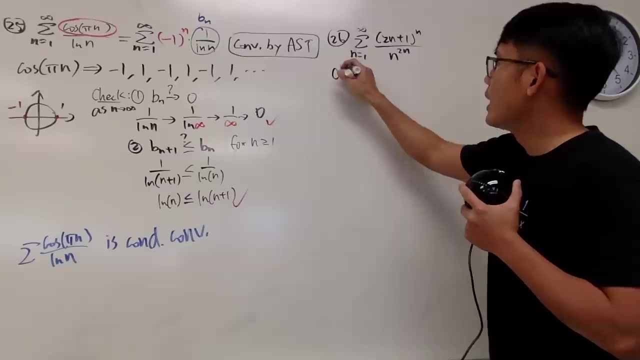 over n to the 2nth power. You can try to do the ratio test, but I will choose the root test because n in the power, n in the power and there's no factorial, so maybe the root test will be the way to go. So here we go. We are going to check as n goes to infinity. 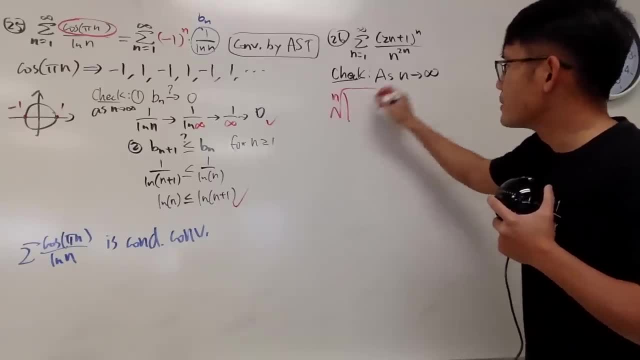 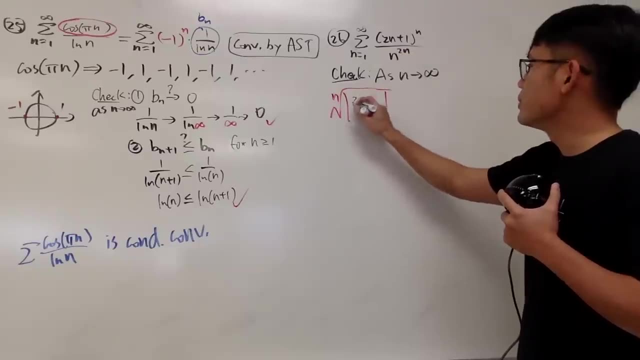 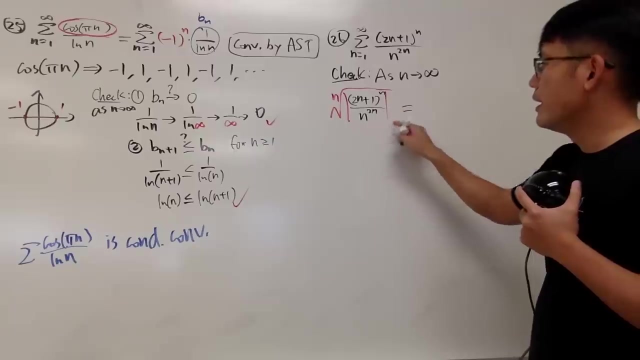 and we are going to open an nth root with an absolute value inside, just in case, with negative terms, inside right. And here we put on the things inside, just this, which is 2n plus 1 to the nth power, over n to the 2nth power, like this: And now remember, when you take the 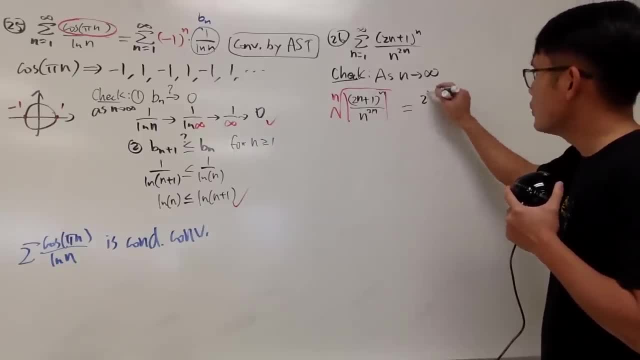 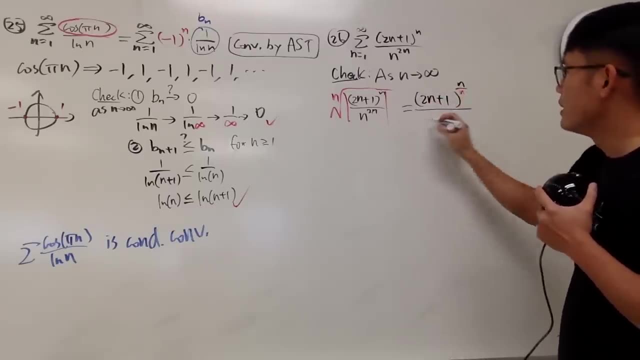 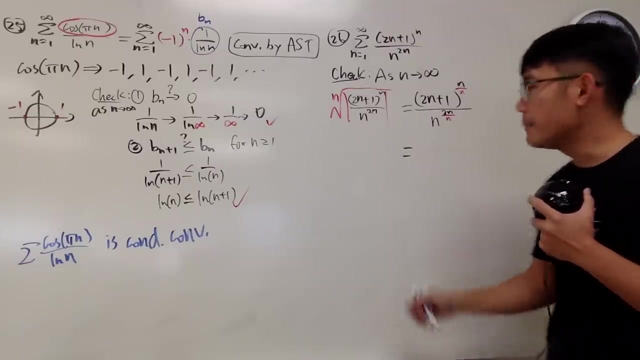 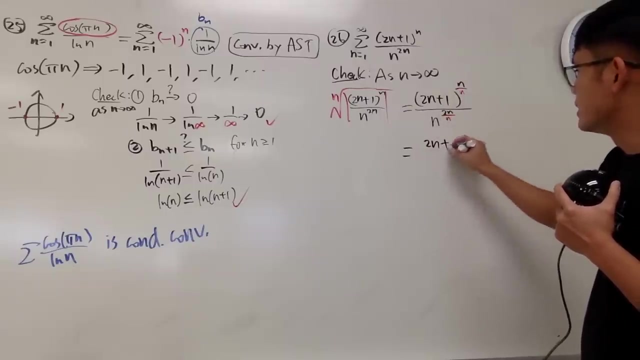 nth root. you just divide the power by n. So we have 2n plus 1 to the n over nth. power over this is n to the 2n, and we divide this by n as well. So, of course, cancel things out. We will end up this right here is just 2n plus 1, yeah. 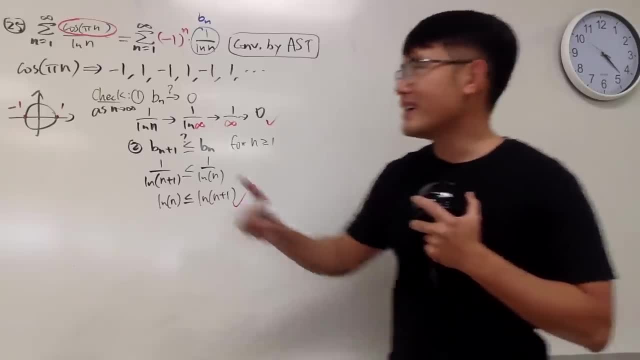 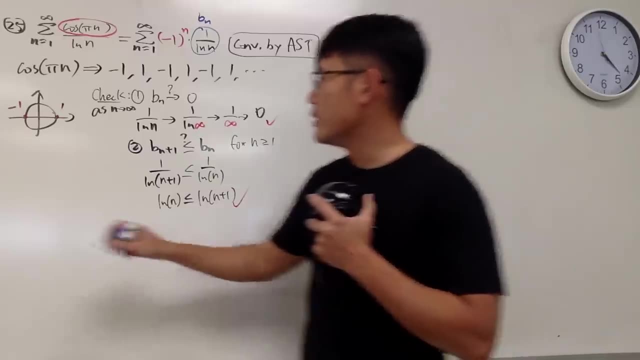 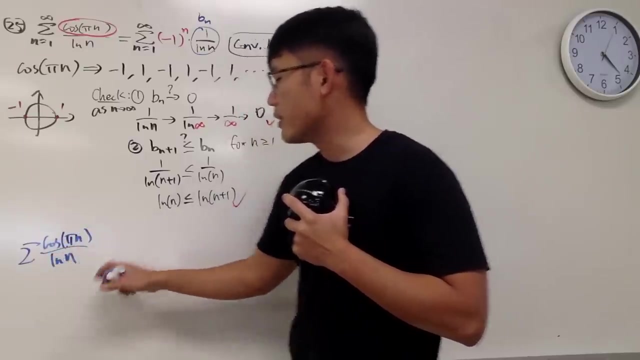 cosine of pi n And again, if you take the absence value, unfortunately this right here does not converge absolutely. So I will just tell you this right here: The sum as cosine of pi n ln n right here is conditional convergent right, Because if you 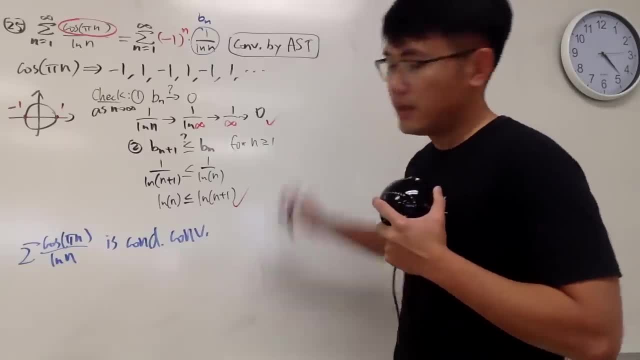 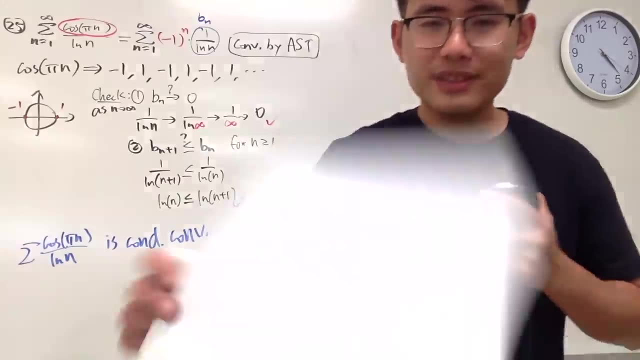 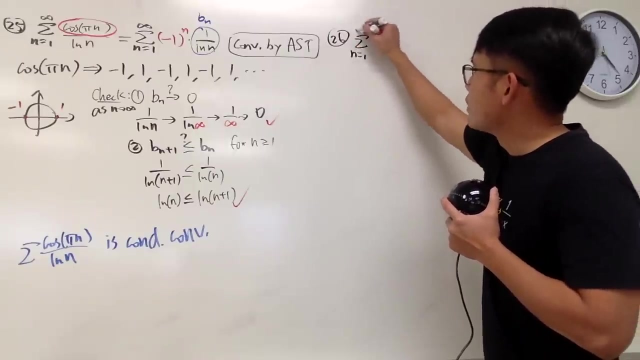 take the absence value, it does not work, It does not converge. Okay, so that's the idea. Now, moving on to hopefully another easy one, Number 26. 26. Here we have the sum as n goes from 1 to. 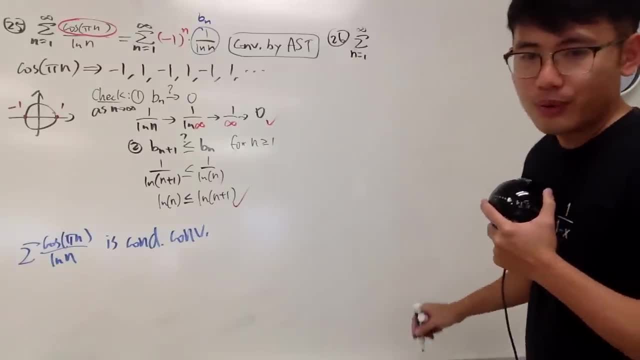 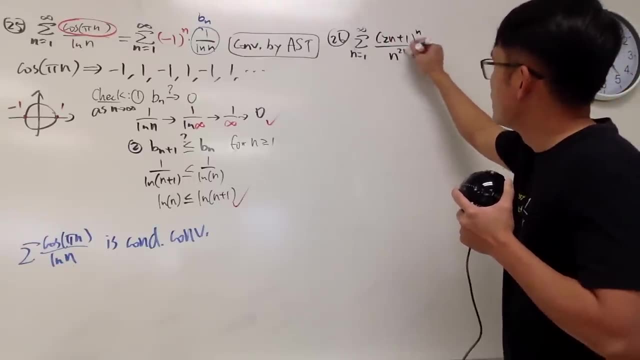 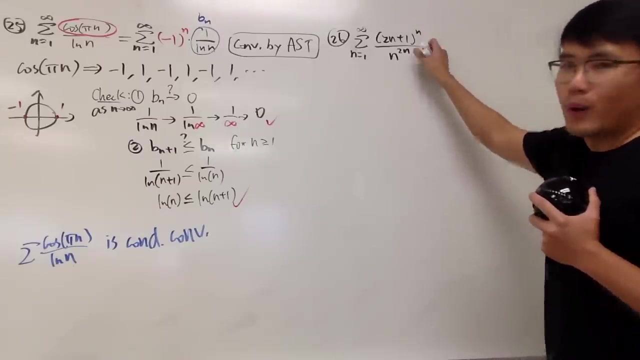 infinity and we are going to have 2n plus 1 to the nth power over n to the 2nth power. Hmm, You can try to do the ratio test, but I will choose the root test because n in the power, n in the power and there's 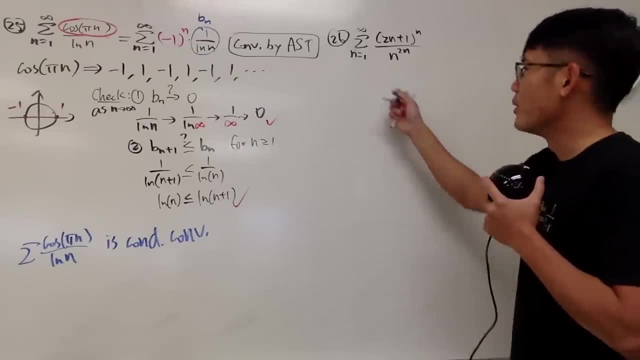 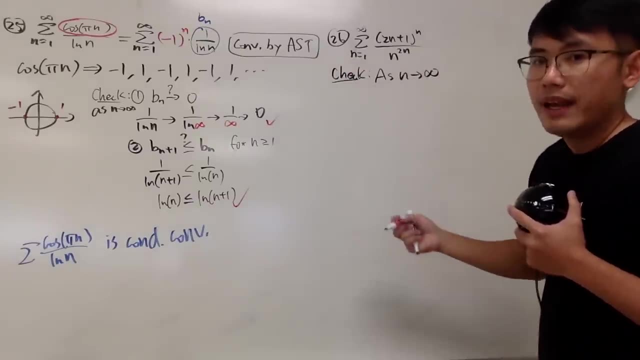 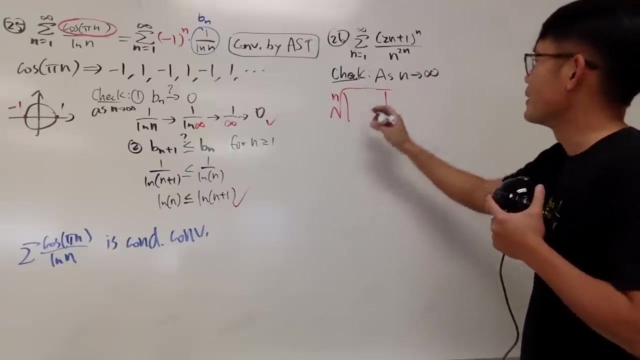 no factorial, so maybe the root test will be the way to go. So here we go. We are going to check as n goes to infinity and we are going to open an nth root with an absence value inside, just in case, with negative terms inside, right? 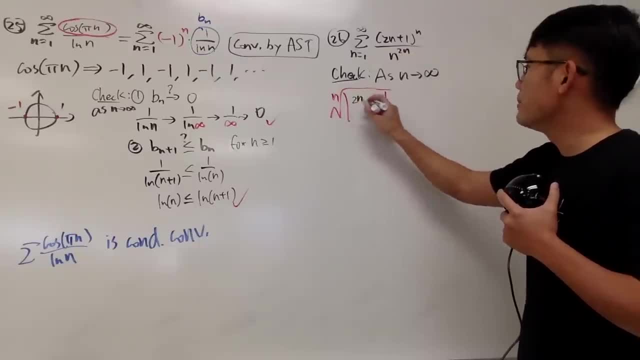 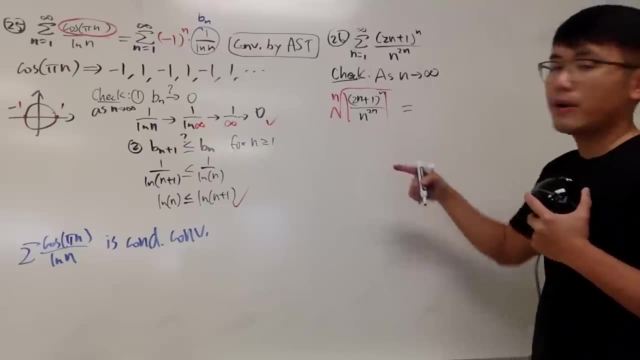 And here we put down the same thing inside just this, which is 2n plus 1 to the nth power, over n to the 2nth power, like this: And now remember, when you take the nth root, you just divide the power by n. 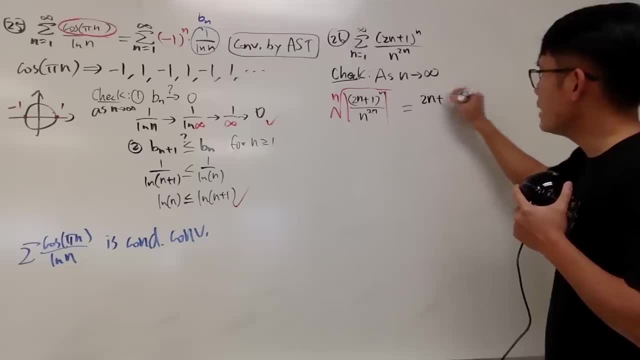 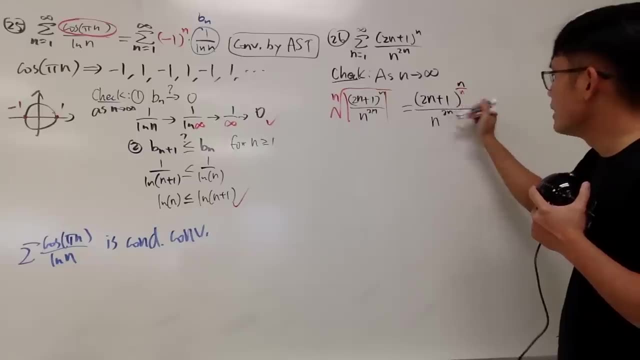 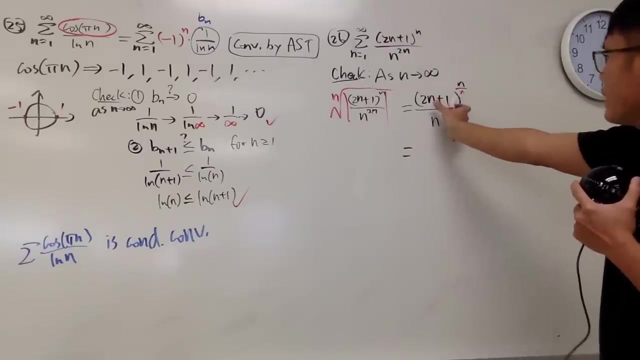 So we have 2n plus 1 to the n over nth. power over this is n to the 2n, and we divide this by n as well. So, of course, cancel things out. We will end up this right here is just 2n plus 1. 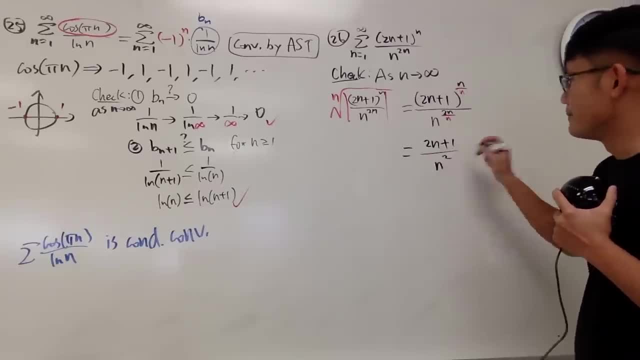 to the first power. and this right here is n squared like that. Take a look what happens as n goes to infinity. You care about this, you care about that. If you work out a limit, this right here does give you 0.. 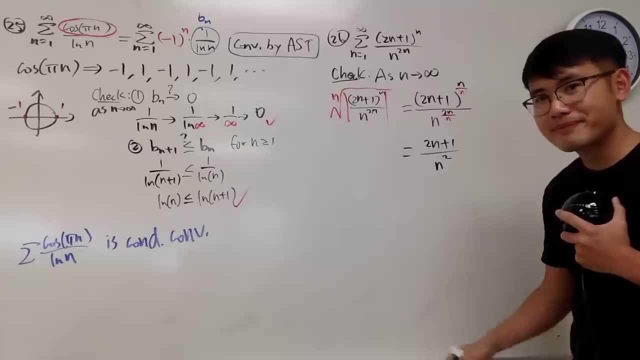 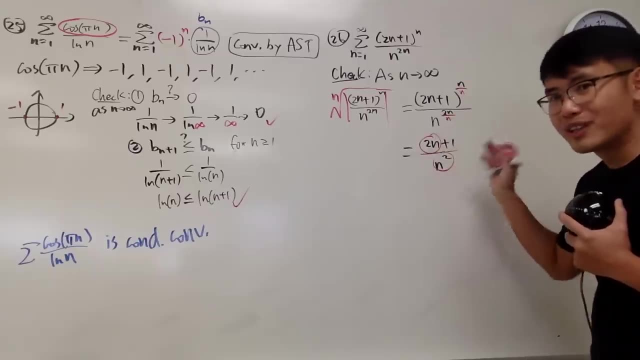 to the first power. and this right here is n squared like that. Take a look What happens as n goes to infinity. You care about this. you care about that. If you work out a limit, this right here does give you. 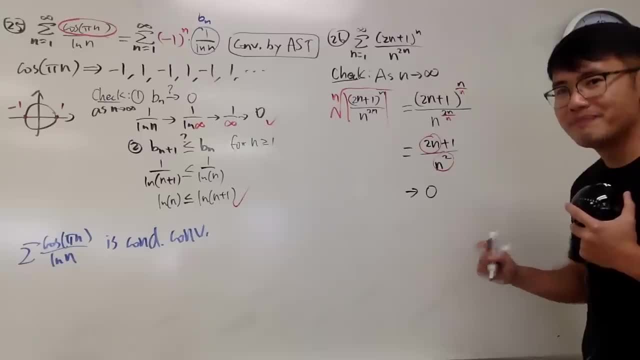 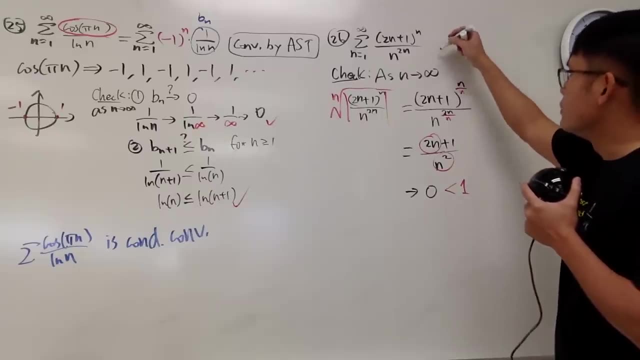 0. And for the root test, does 0 help? Yes, it does. It's less than 1, right? So this right here we can come up and draw a conclusion. This right here actually converges by the root test. 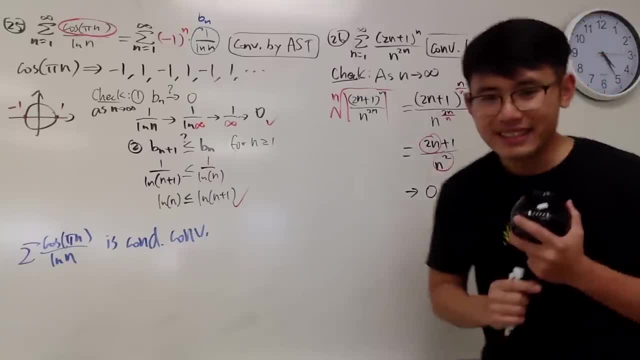 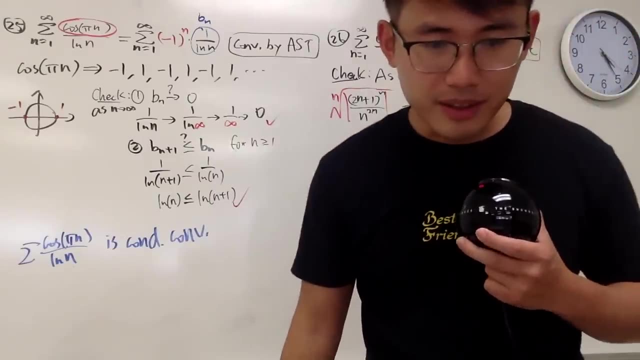 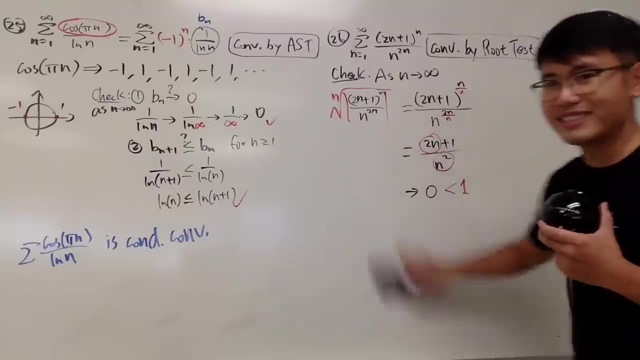 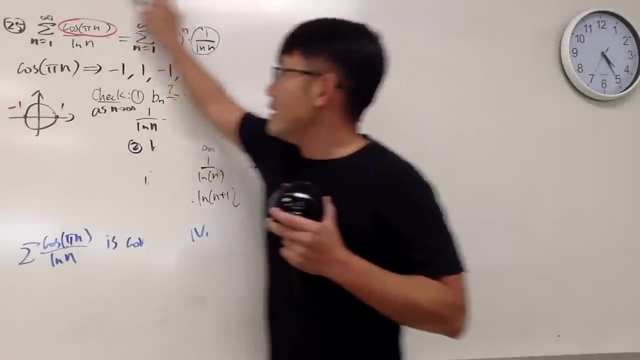 Done, okay, Done, Okay, Number 27.. Number 27.. Okay, I have to do number 27 and number 28 side by side, so I will erase all this. I don't know if I can finish this in six hours or not. This is like amazingly hard. 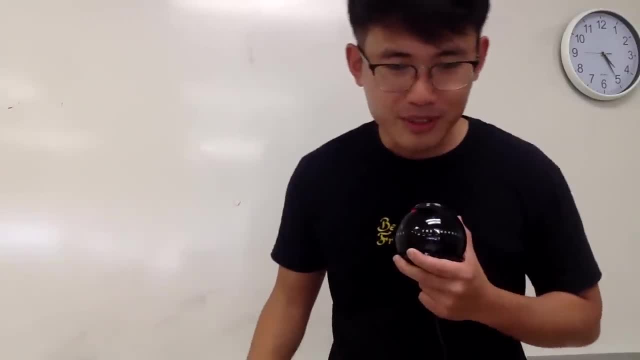 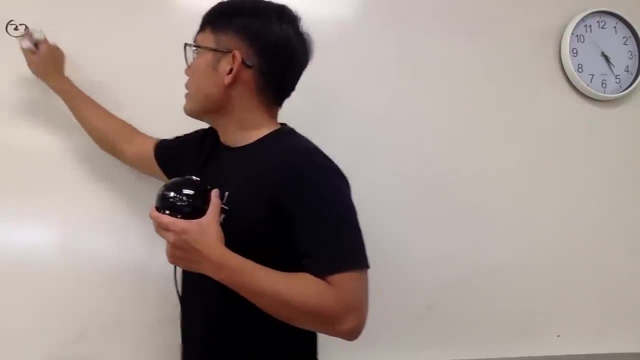 Didn't expect to be this long. I'm trying to provide the most to the just now. I'm just going to focus, Anyway, number 27.. Here is the sum as n goes from. we want to do 1.. Okay, 1 is okay in this case. 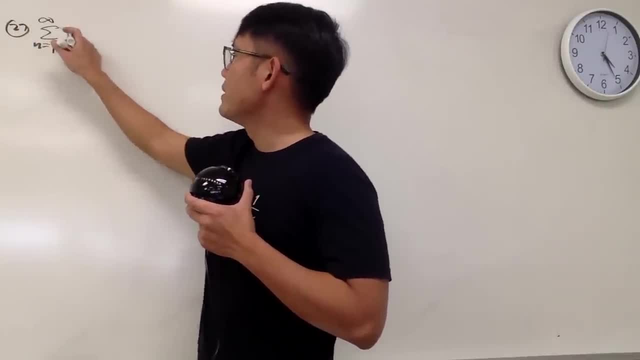 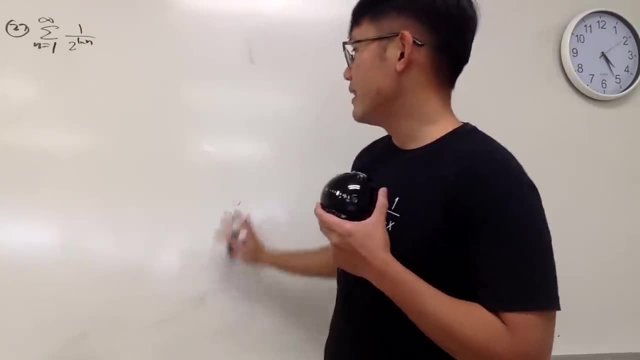 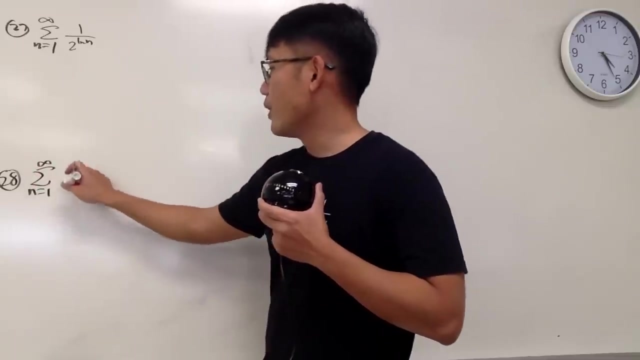 1 to the 1 and n to infinity, and then, right here, 2 to the natural log of n. Wow, And as I said, I will do 28 right here as well. This is the sum as n goes from 1 to infinity, 1 over 3 to the natural log of n. 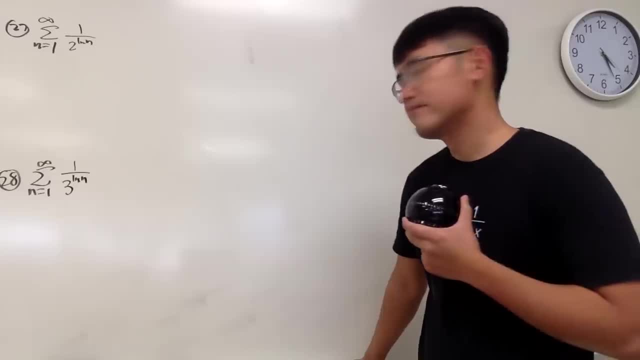 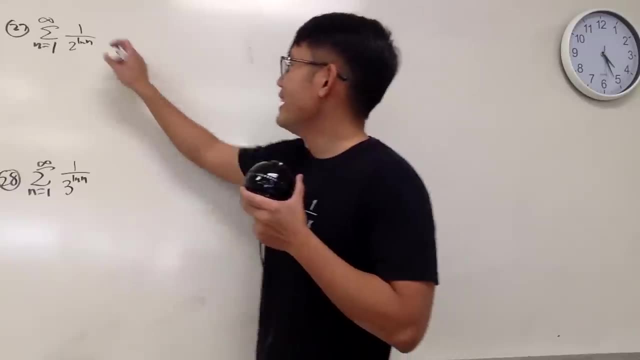 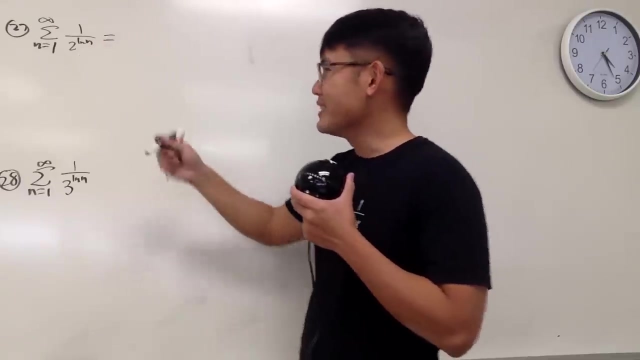 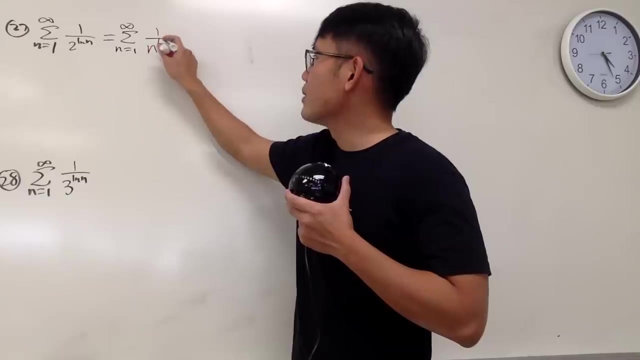 What should we do? Well, let me just impress you guys a little bit. The truth is base and the input of the natural log can be switched. So, in other words, this right here is actually the sum as n goes from 1 to infinity of 1, over n to the natural log of 2 power. 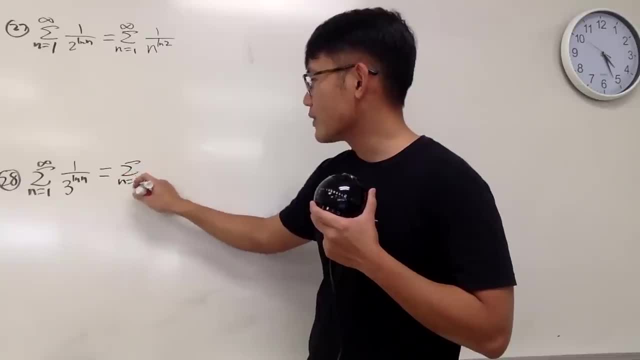 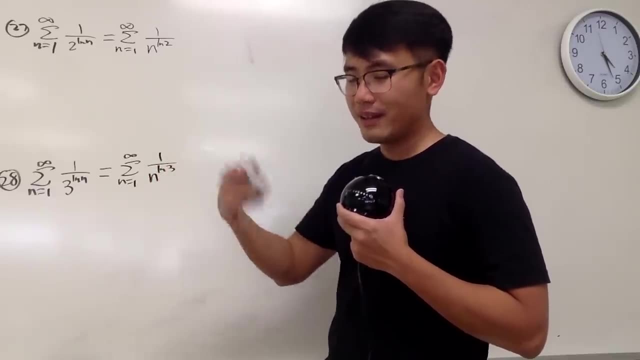 Similarly right here. this is actually the sum, as n goes from 1 to infinity, of 1 over n to the natural log of 3 power. We did that, like in the earlier question, right, And perhaps I'll do a quick proof again right here. 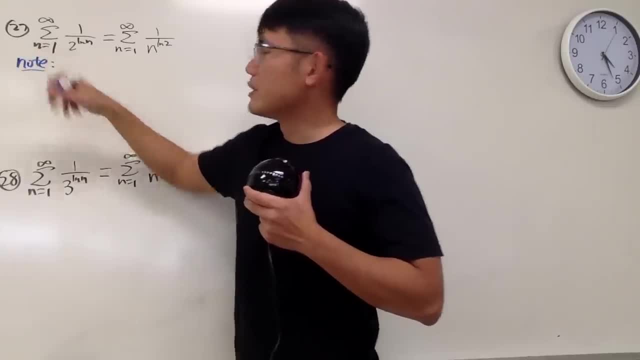 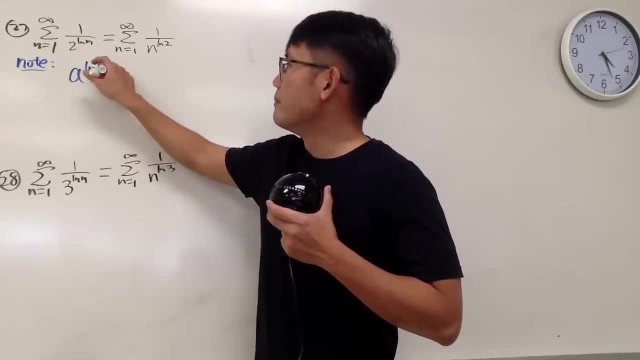 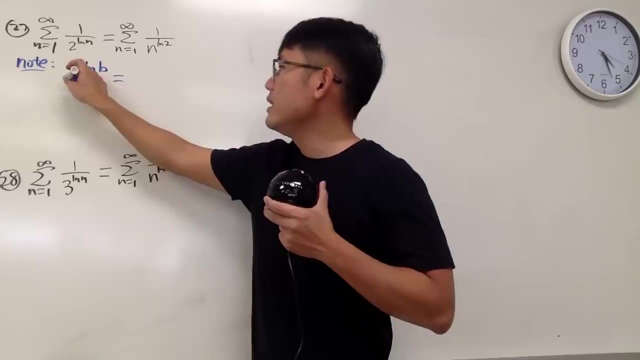 So here is the proof for that property. I'll just put this down in general. So suppose we have, let's say, a to the natural log of b's power like that. Well, in this case, we don't like to have base a, we like to have base e, so it's okay. 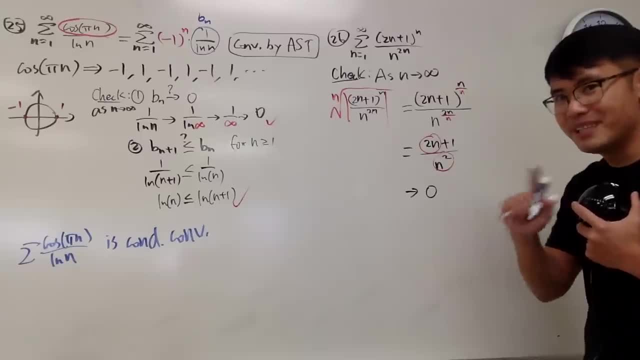 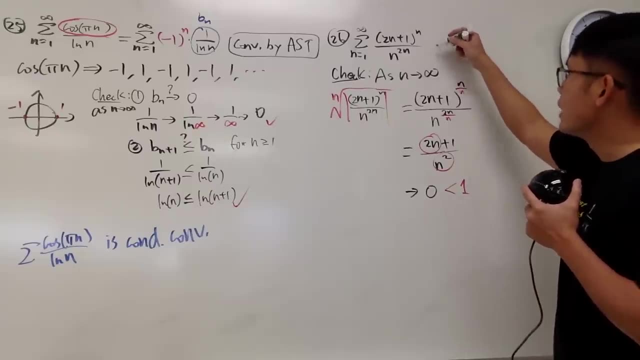 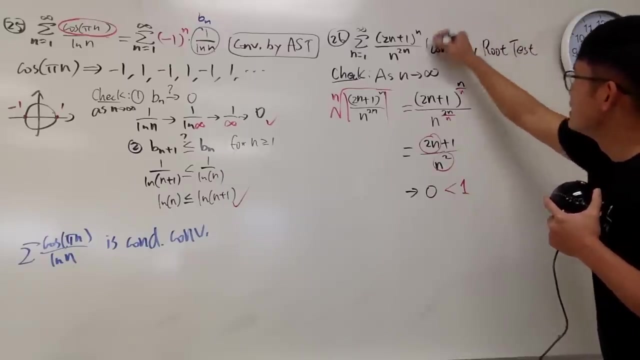 And for the root test: does 0 help? Yes, it does, It's less than 1.. Right, So this right here we can come up and draw a conclusion. This right here actually converges by the root test Done. 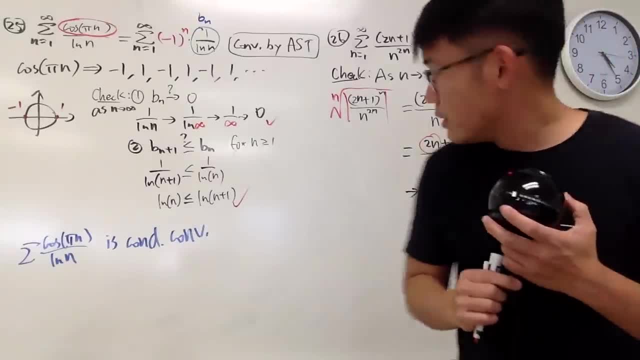 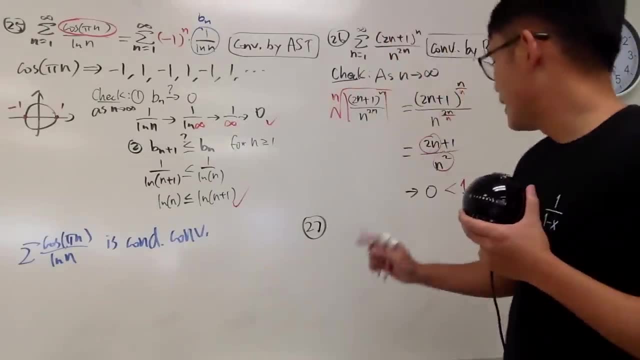 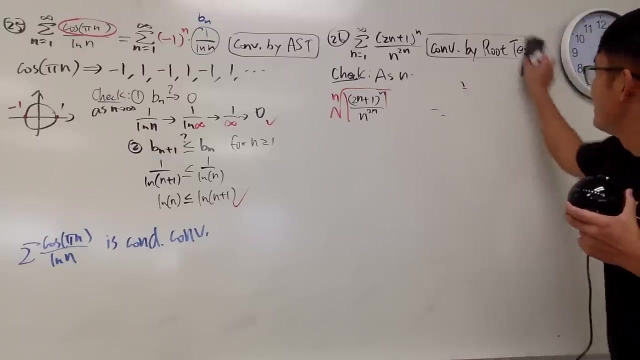 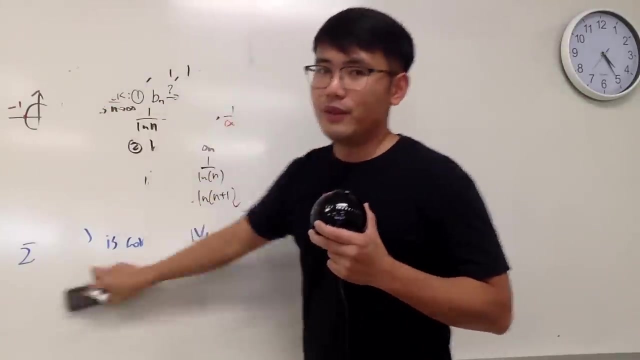 Okay, Done. Okay. Number 27.. Number 27.. Okay, I have to do number 27 and number 28 side by side, so we'll erase all this. I don't know if I can finish this in 6 hours or not. 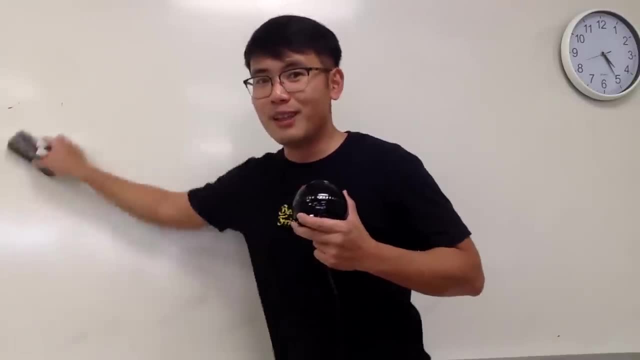 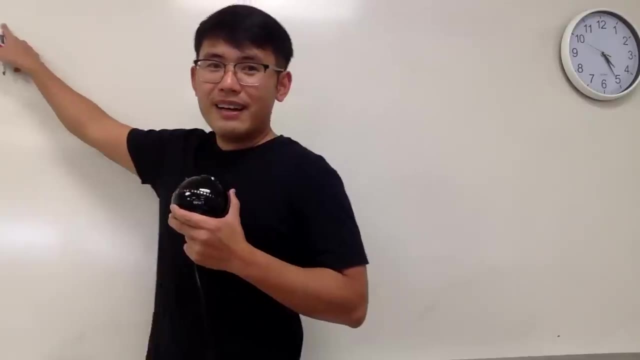 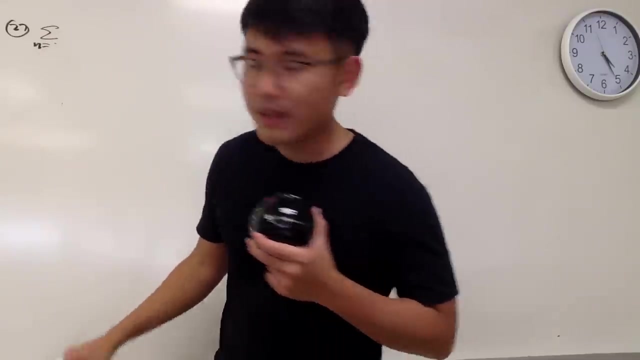 This is like amazingly hard. Didn't expect to be this long. I'm trying to provide the most to the. I'm just gonna focus, Anyway. number 27.. Here is the sum as n goes from. we want to do 1.. 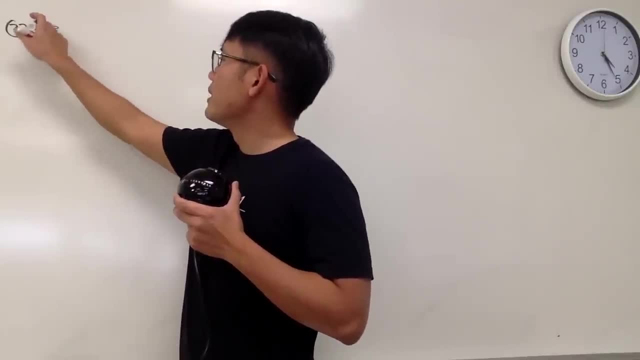 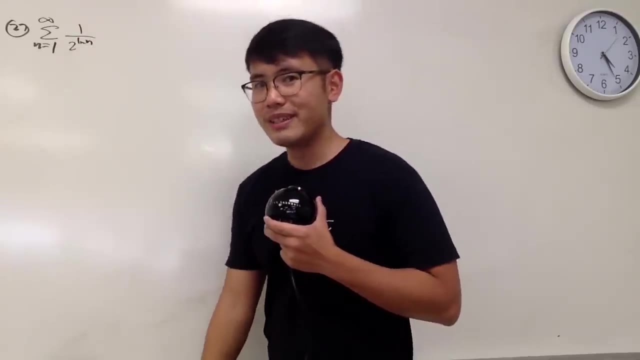 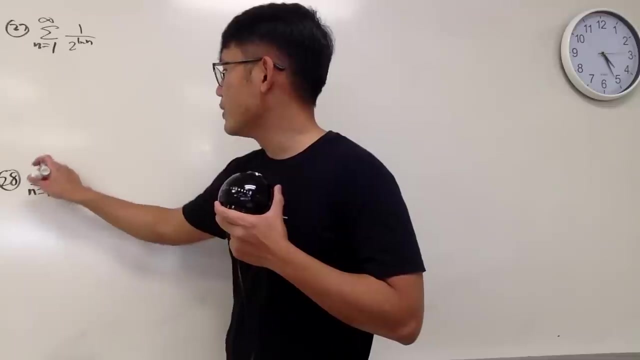 1 is okay in this case, 1 to infinity, and then, right here, 2 to the natural log of n. Wow, And as I said, I will do 28 right here as well. This is the sum as n goes from 1 to infinity. 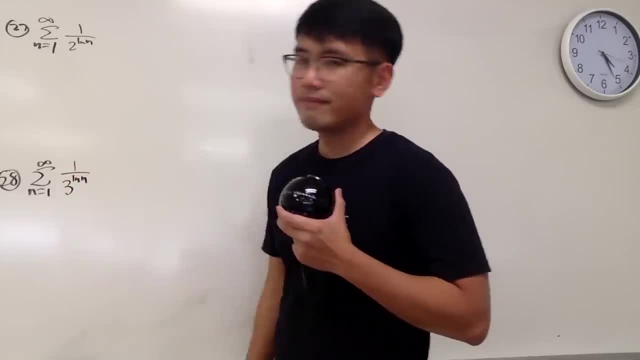 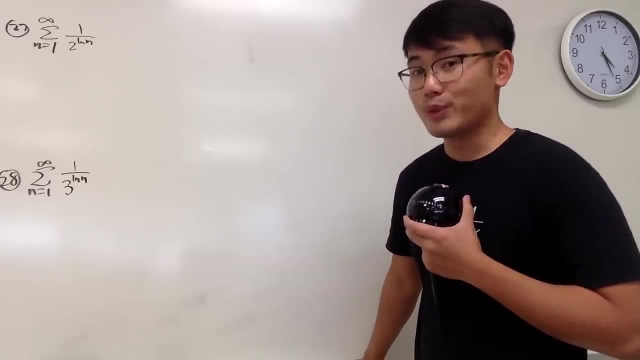 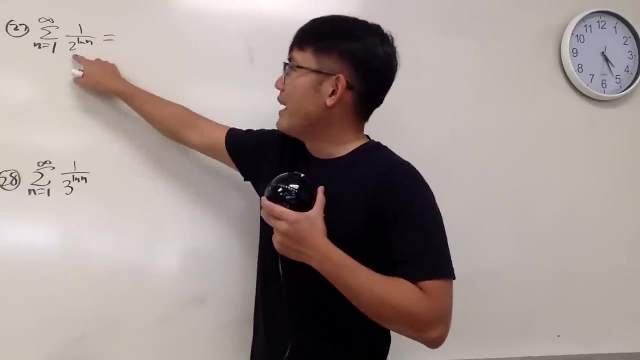 1 over 3 to the natural log of n. Hmm, What should we do? Well, let me just impress you guys a little bit. The truth is base and the input of the natural log can be switched. So, in other words, this right here is actually the sum. 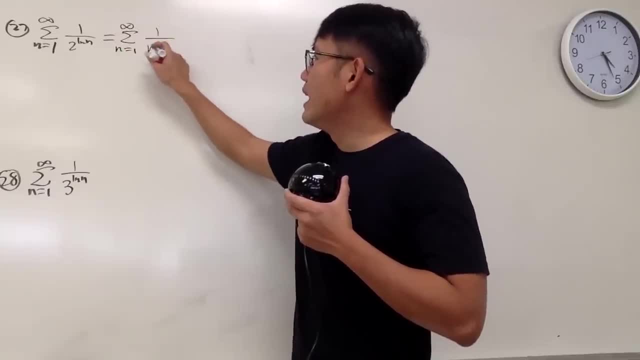 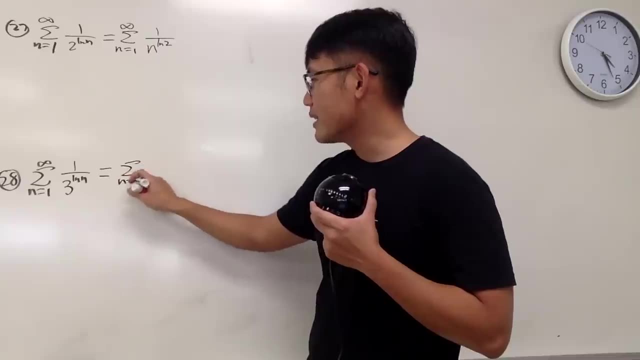 as n goes from 1 to infinity of 1 over n to the natural log of 2 power. Similarly, right here, this is actually the sum as n goes from 1 to infinity of 1 over n to the natural log of 3. 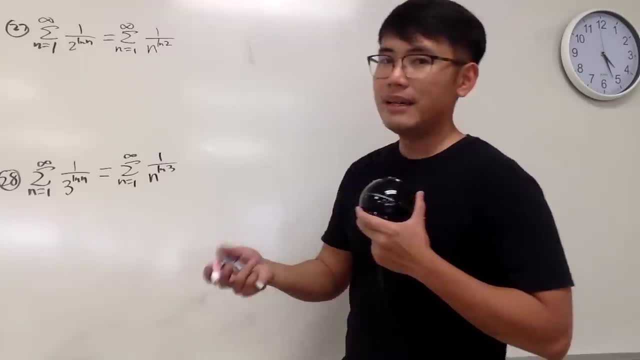 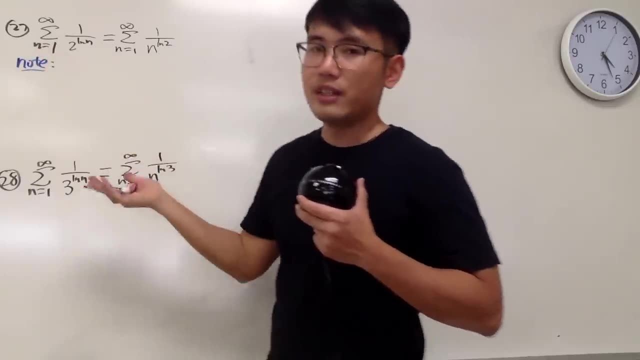 power. We did that in the earlier question, right, And perhaps I'll do a quick proof again right here. So here is the proof for that property. I'll just put this down in general. So suppose we have, let's say, a to the natural. 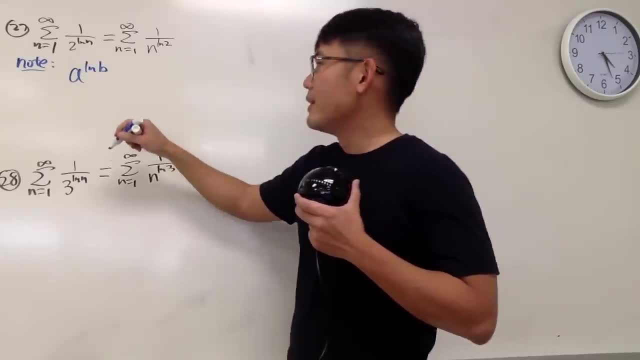 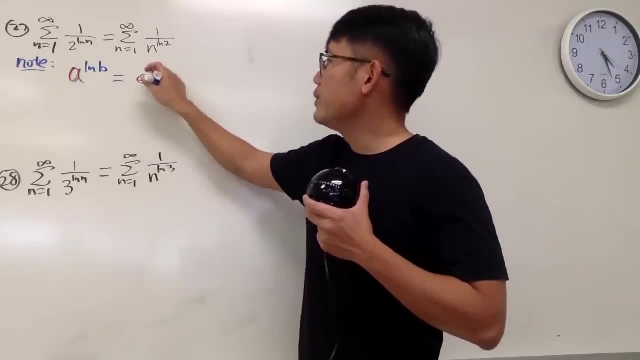 log of b's power like that. Well, in this case we don't like to have base a, We like to have base e. So it's okay, We look at a as e to the natural log of a's power, and then we will just look at this. 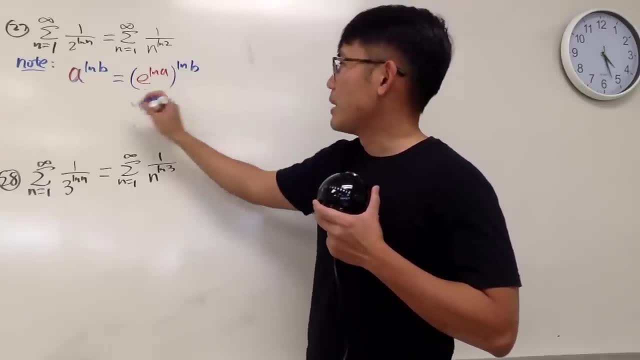 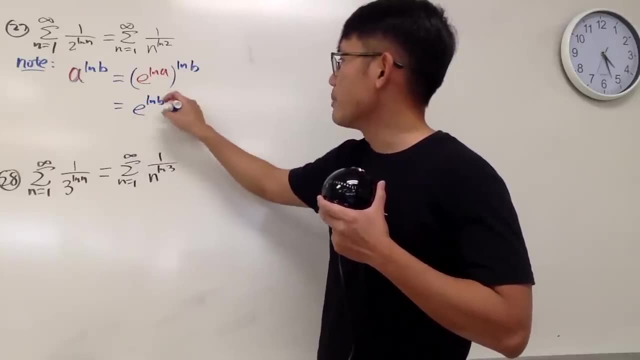 as natural log of b's power, like this, And again we can multiply the powers, and we can look at this as e and then multiply this and that. So I'll put down ln b first and then multiply by ln a, And again we can write. 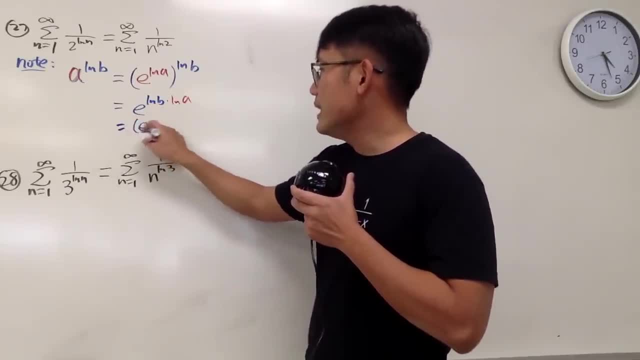 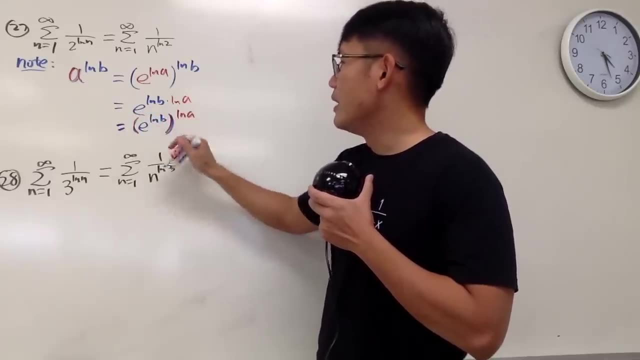 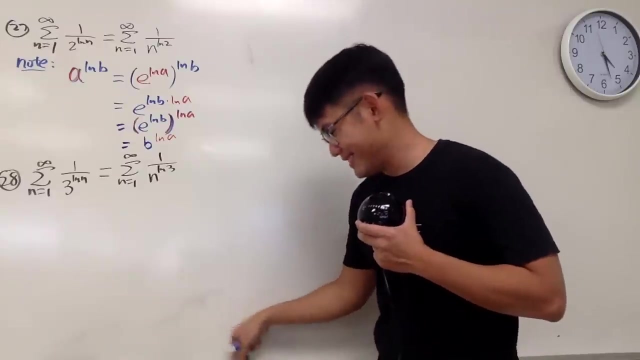 this down for the base, which is parentheses e to the ln b, and then we raise this to the ln a's power And of course you can see that inside now is just b and outside now is just ln a. Cool huh. 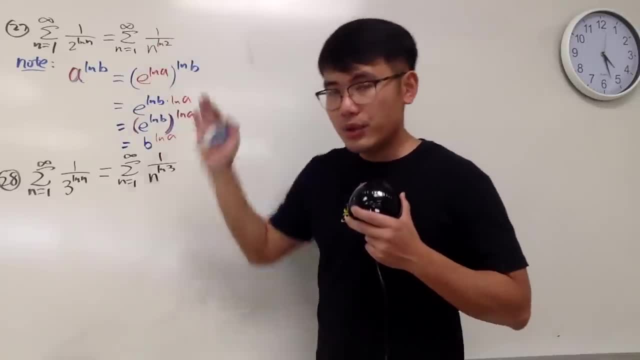 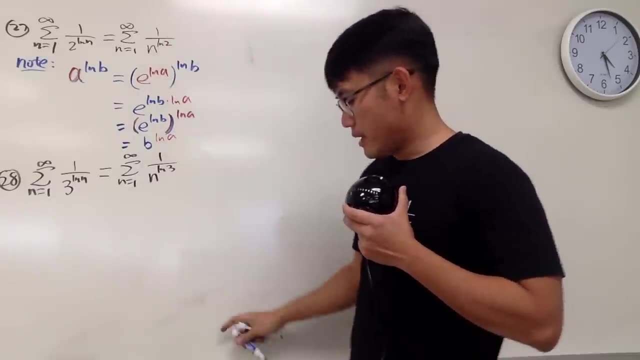 Okay, now here's the deal. ln 2 is a constant, so we can just use the p-series for this: 1 over n to the p's power, And you have to just kind of know some famous numbers, of course. 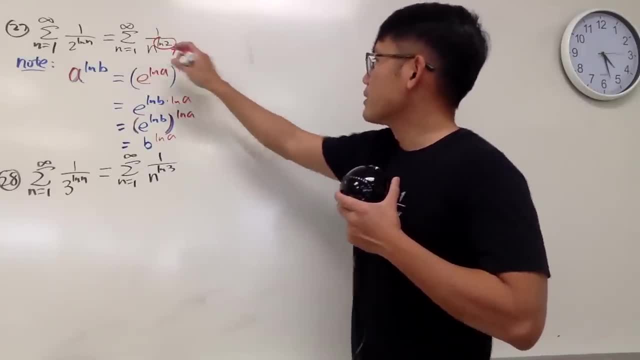 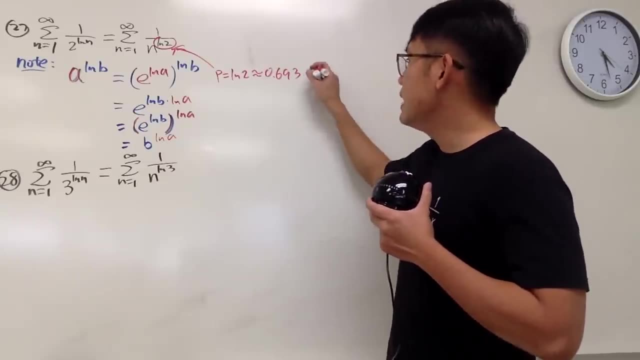 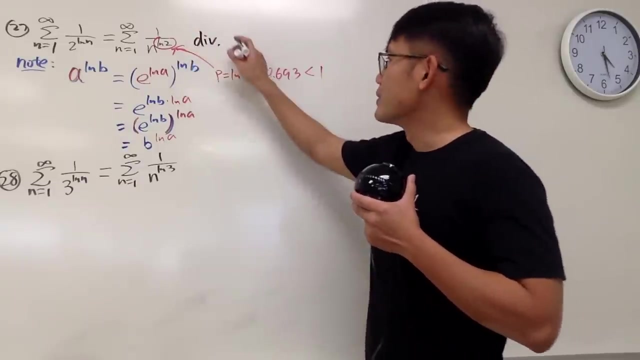 I will just put this down right here: In our situation, p is ln 2,, which is approximately 0.693, and in this case is less than 1. So this right here in fact diverges. Right, I'll just say diverges. 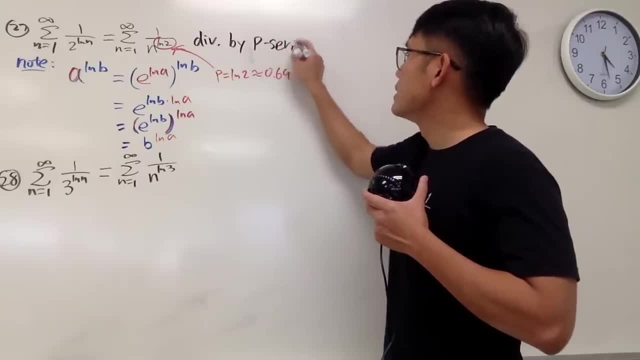 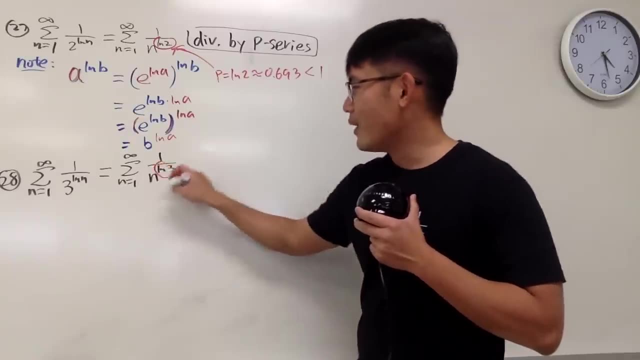 by the p-series. Right Diverges by p-series? Well, on the contrary, right here we have ln 3 for the p. so I'll just put down: p is equal to ln 3 and this right here is bigger than. 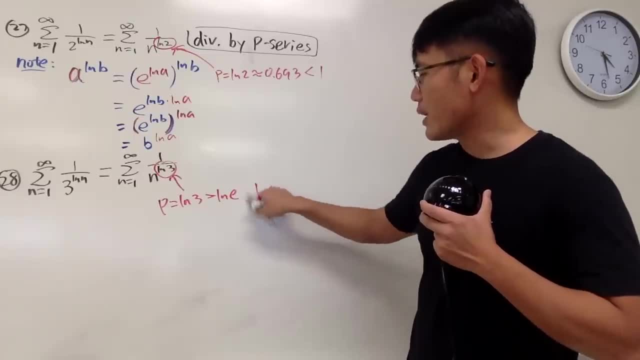 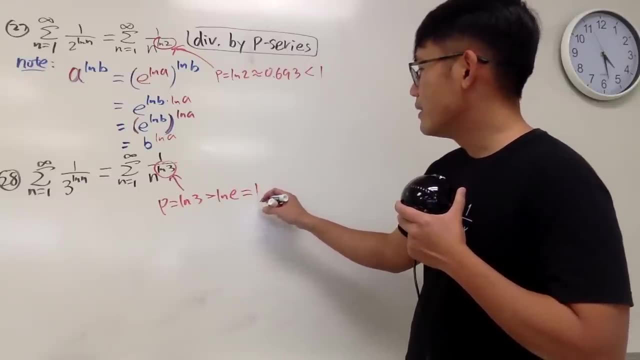 ln e, which is bigger than 1.. ln e is equal to 1.. So, all in all, we have: ln 3 is bigger than 1, and, of course, if the p is bigger than 1, yeah, p is bigger than 1, right. 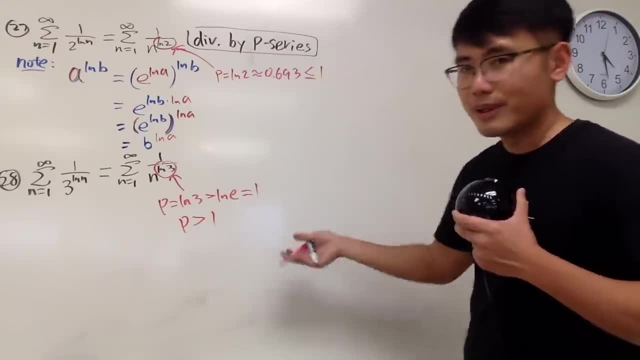 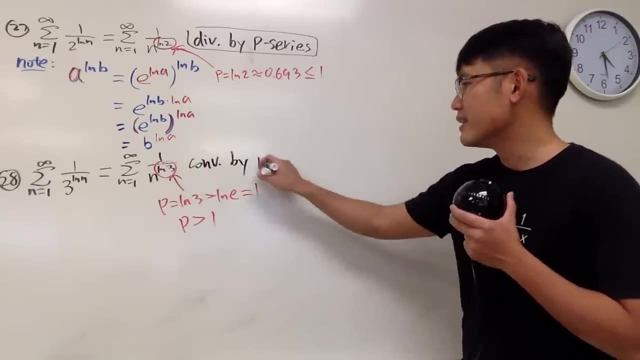 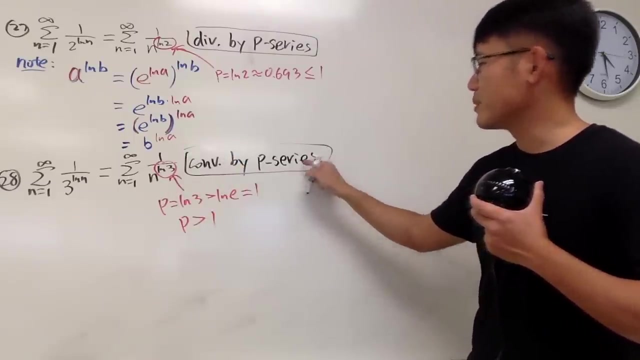 This: right here p is bigger than 1, that means this right here converges by p-series again. Well, p-test, p-series, up to you. I think both are okay. I usually call this the p-series or the p-test, up to you. 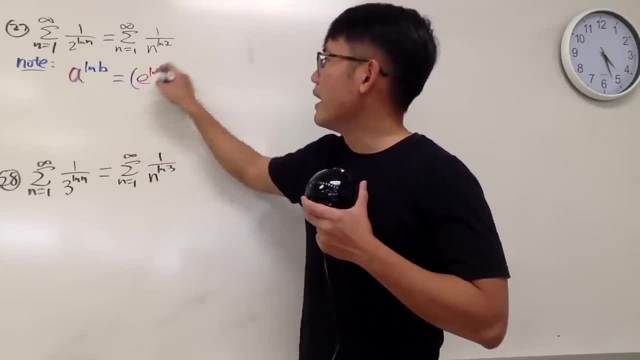 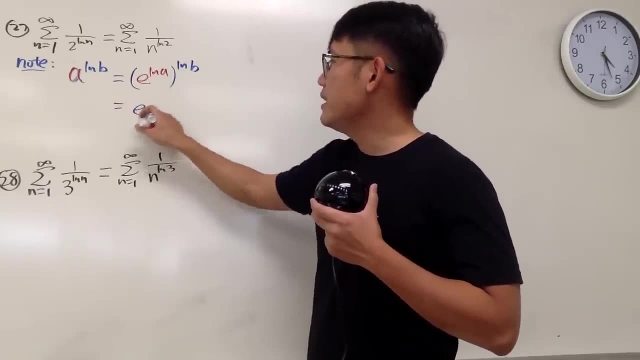 We look at a as e to the natural log of a's power, and then we will just look at this as natural log of b's power, like this. And again, we can multiply the powers and we can look at this as e and then multiply this and that. 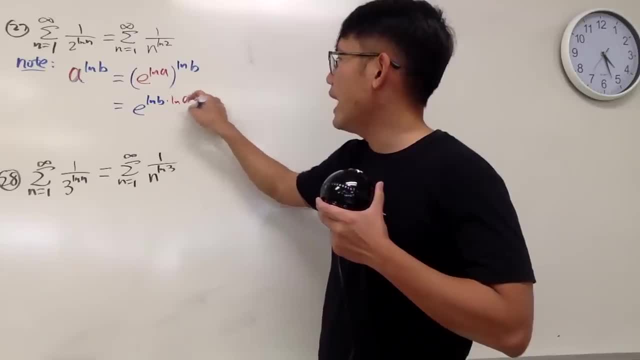 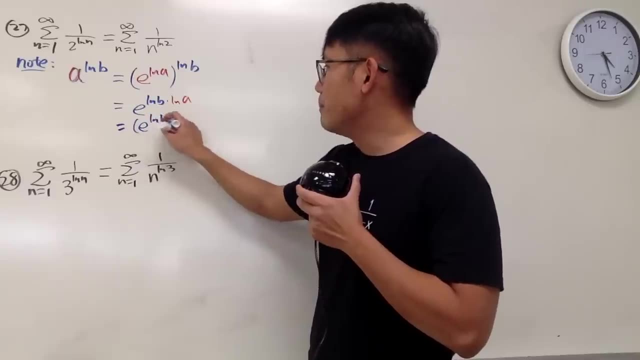 So I'll put down ln b first and then multiply by ln a, And again we can write this down for the base, which is parentheses e to the ln And b, and then we raise this to the ln a's power. 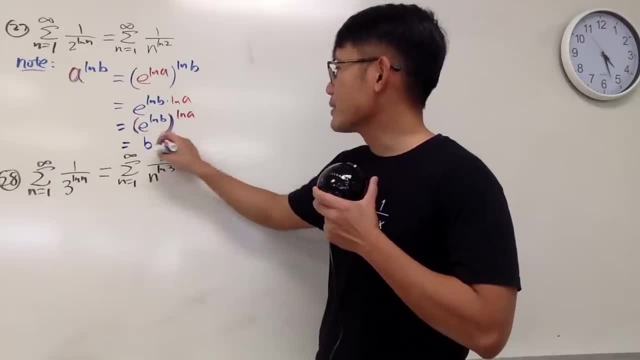 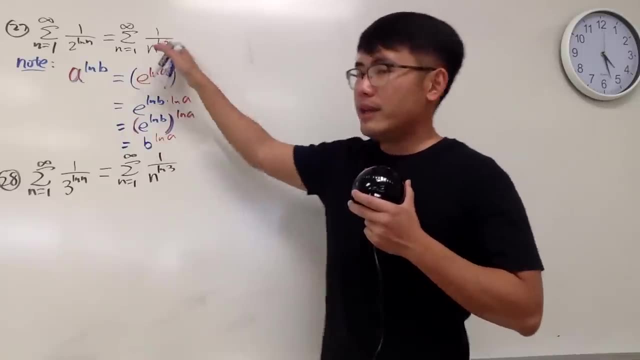 And of course you can see that inside now is just b and outside now is just ln a. Cool huh. Okay, now here's the deal. ln 2 is a constant, so we can just use the p-series for this. 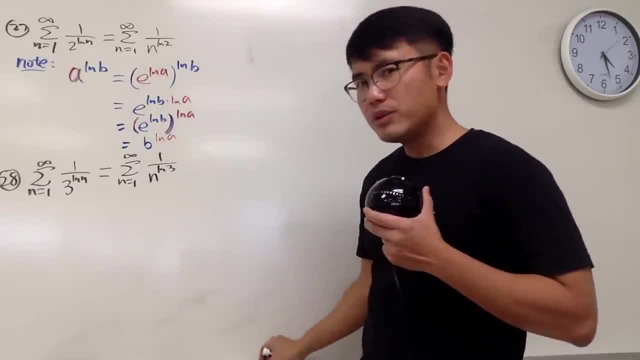 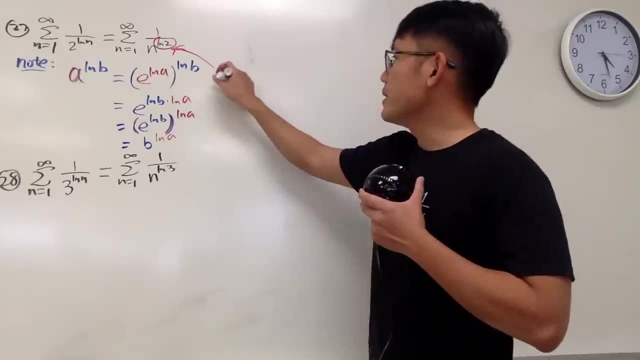 1 over n to the p's power, And you have to just kind of know some famous numbers, of course. I will just put this down right here: In our situation, p is ln 2, which is approximately 0.693.. 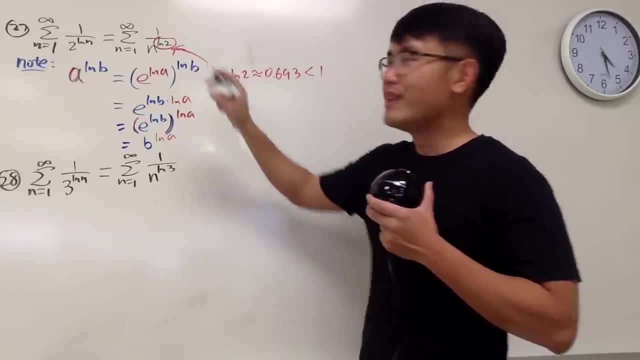 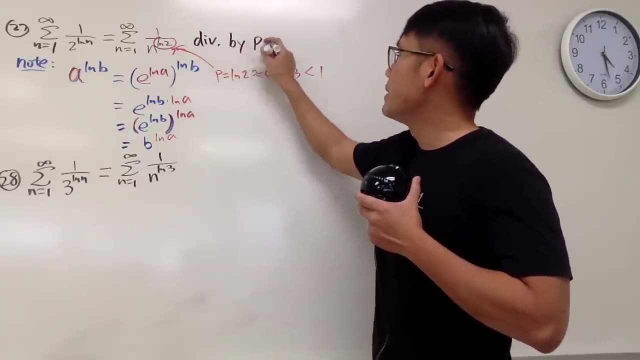 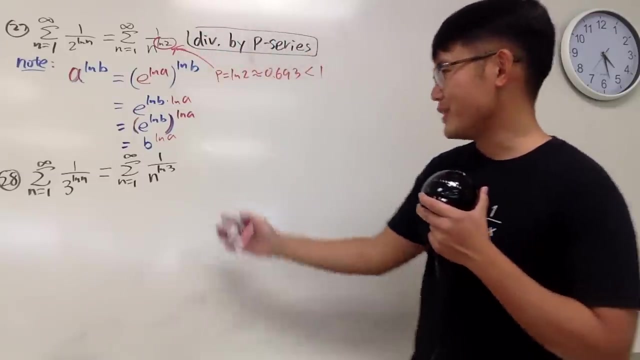 And in this case it's less than 1.. So this right here in fact diverges, Right, I'll just say diverges by the p-series. Right, Diverges by p-series. Well, on the contrary, right here we have ln 3 for the p. 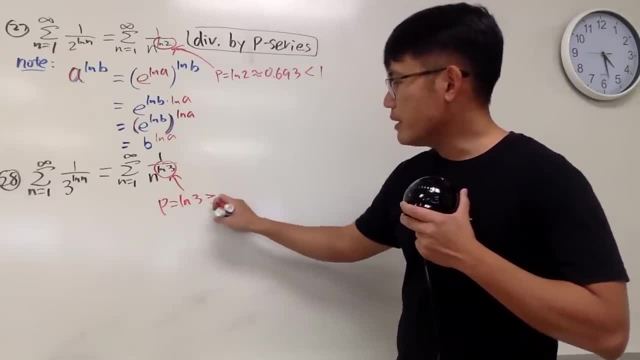 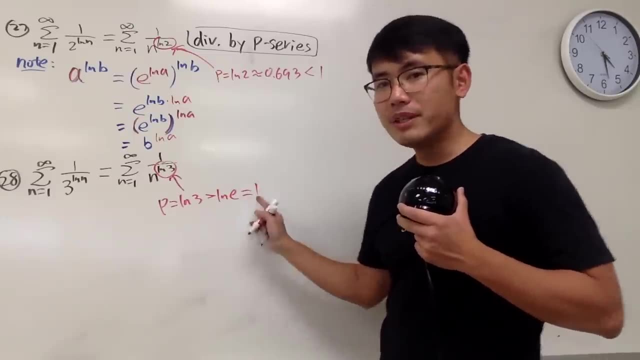 So I'll just put down: p is equal to ln 3. And this right here is bigger than ln e, which is bigger than 1.. Well, ln e is equal to 1.. So all in all we have: ln 3 is bigger than 1.. 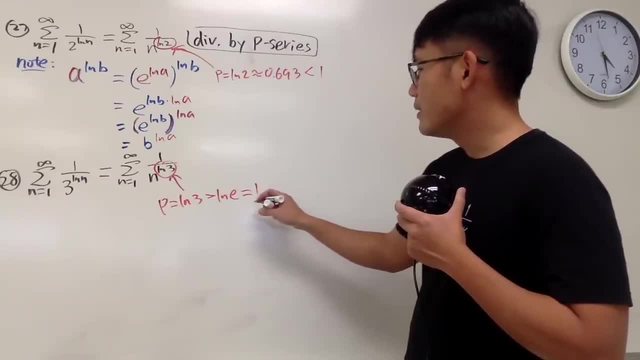 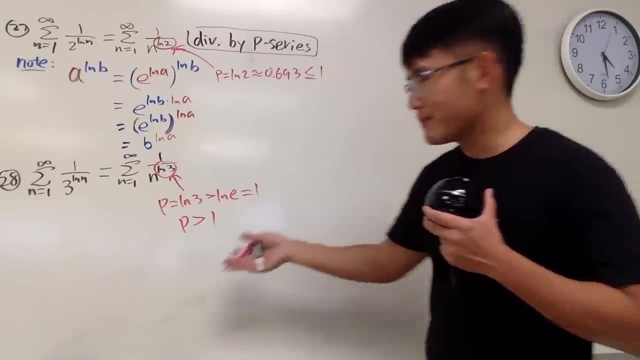 And, of course, if the p is bigger than 1.. Yeah, p is bigger than 1,, right, p is bigger than 1.. This right here, Well, you should have said less than or equal to: yeah, p is bigger than 1,. that means, this right here converges by p-series again. 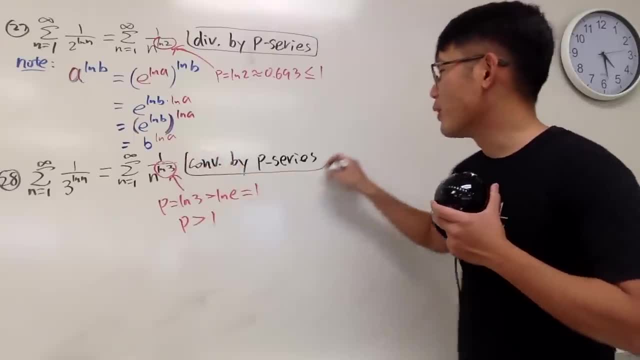 p. Well, p-test, p-series, up to you. I think both are okay. I usually call this the p-series or the p-test, up to you, right? Whichever one you want to use. So these two questions done. 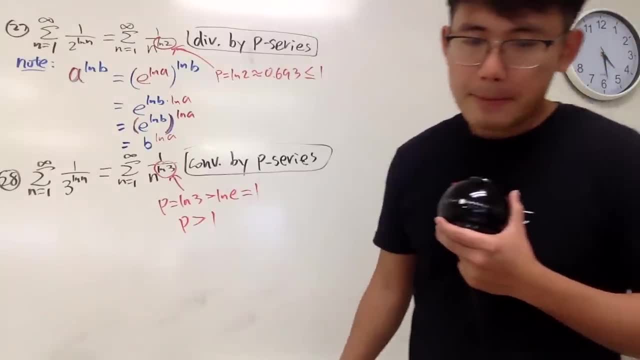 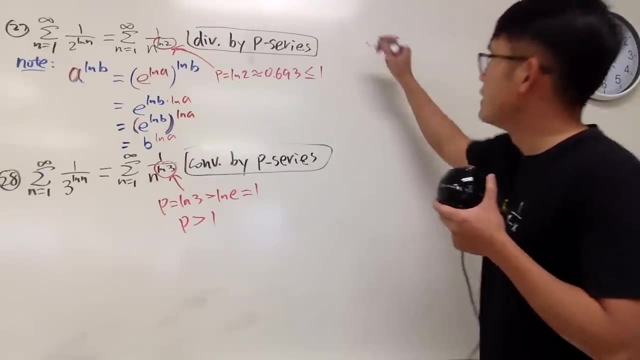 Now let's see, Hmm, Number 29.. This is the one that I will really show the students, like the three steps and all that stuff, So I will put this down. I should be able to fit in here Number 29.. 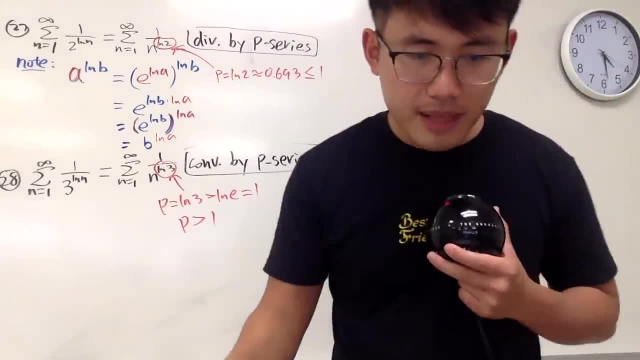 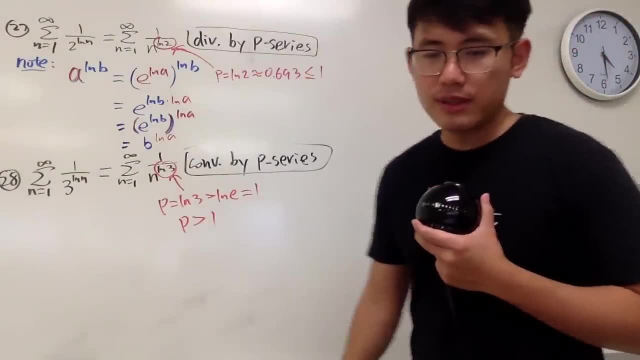 Whichever one you want to use. So these two questions done, Now let's see, Hmm, 29.. This is the one that I will really show the students, like the three steps and all that stuff, So I will put this down. 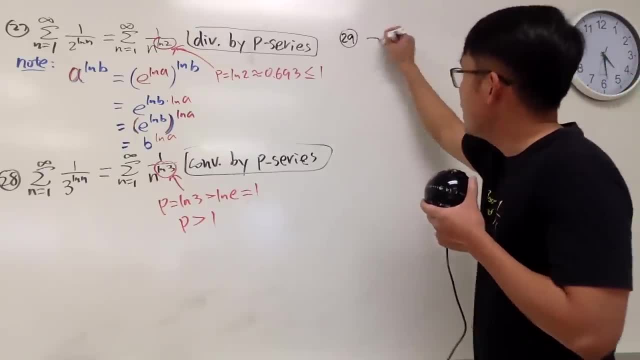 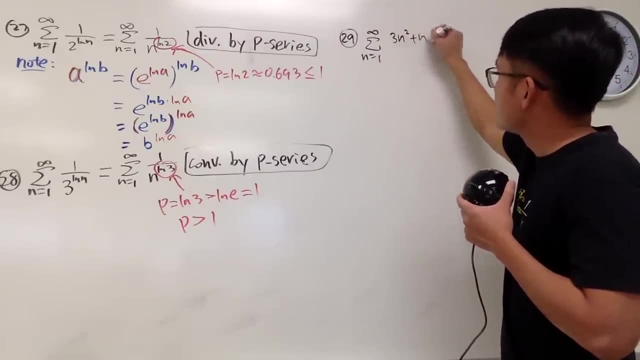 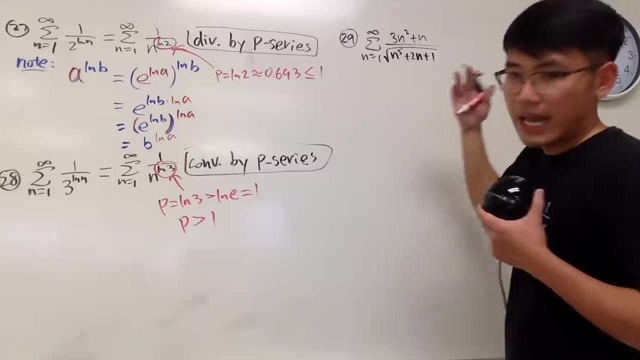 I should be able to fit in here Number 29.. We are going to do the sum as n goes from 1 to infinity, and then we have 3n squared plus n over square root of n to the fifth power, plus 2n plus 1, like this: 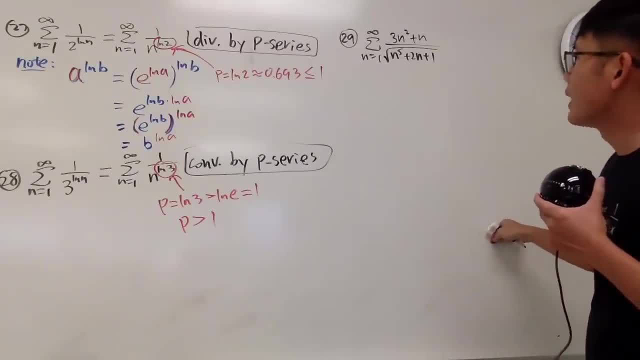 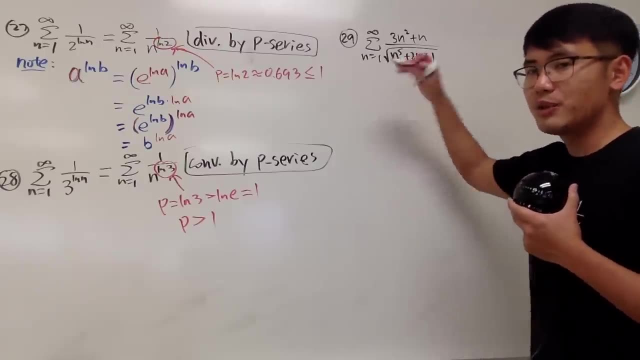 Okay. Well, it's a big rational expression and all that, So I will try to just pick the dominating part. Luckily there's no like weird natural log or whatever, such as like polynomial inside here of the square root. 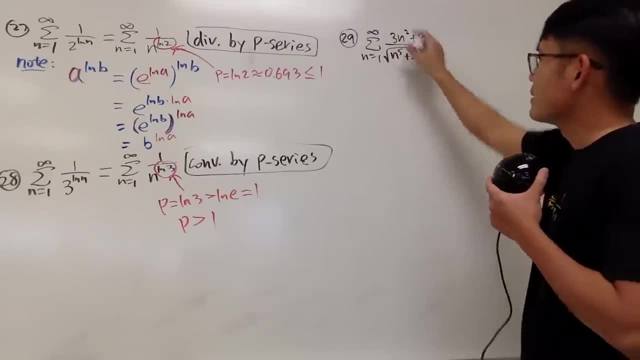 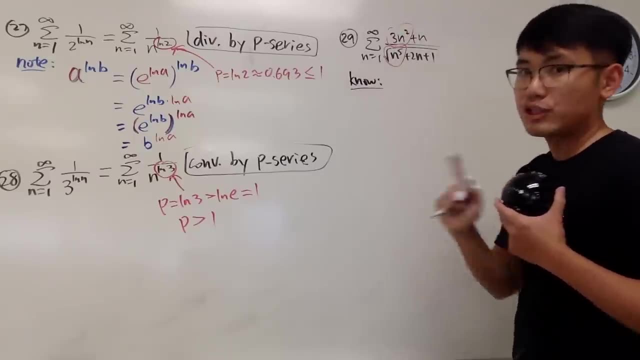 and all that. This is not polynomial because of square root, but I'm saying inside. So just look at the powers, So look at this and look at that, And perhaps this is what we know much better, right? So put down what we know. 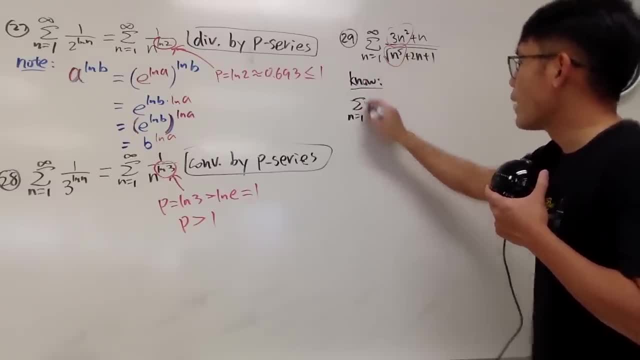 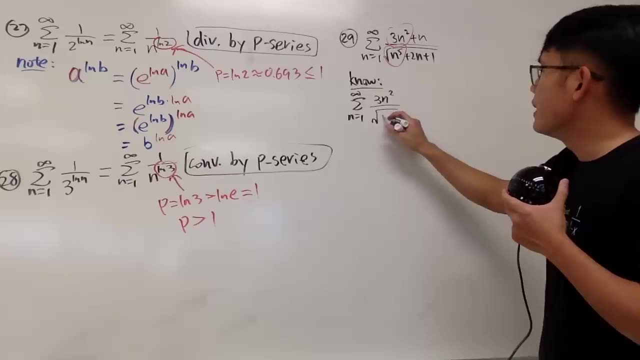 I will just write down the sum as n goes from 1 to infinity, and then here on the top we have 3n squared over square root of n to the fifth power like this: Okay, here's the deal. We can put the 3 in the front. This is a. 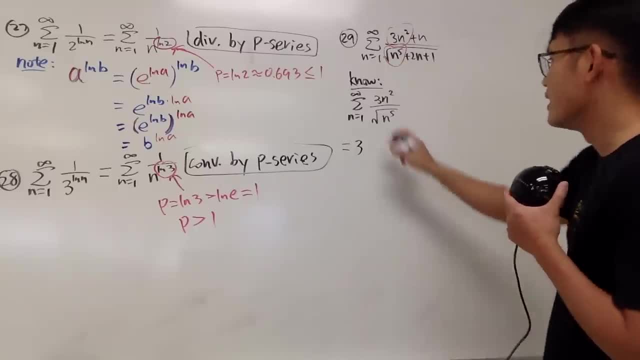 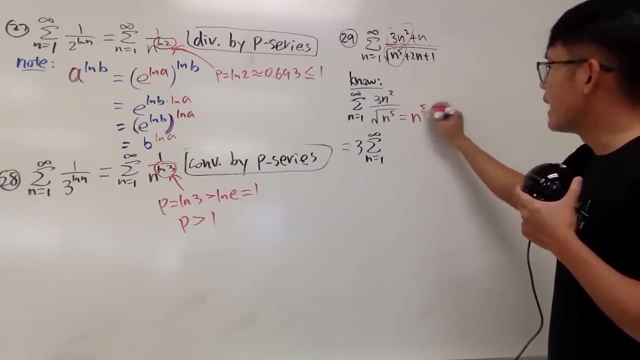 constant multiple. so just that integration. you can take that all the way to the front, that's okay. And then we have the sum, as n goes from 1 to infinity. and notice this right here is like saying n to the 5 over 2 power. 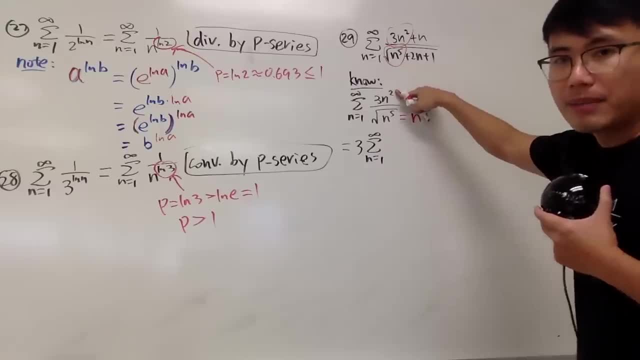 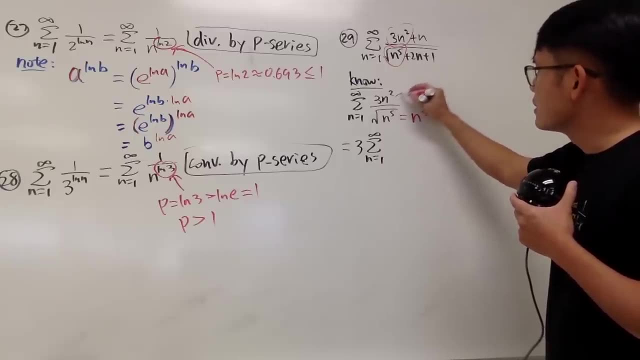 Now, on the top we have 2, and on the bottom we have 5 over 2.. So, in another word, this right here is actually the same as saying n to the 4 over 2, right, So we actually have just n to the. 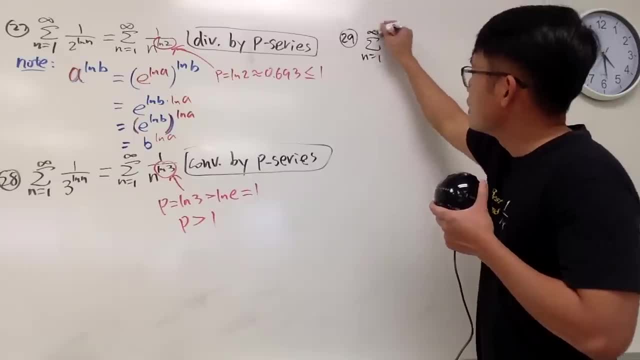 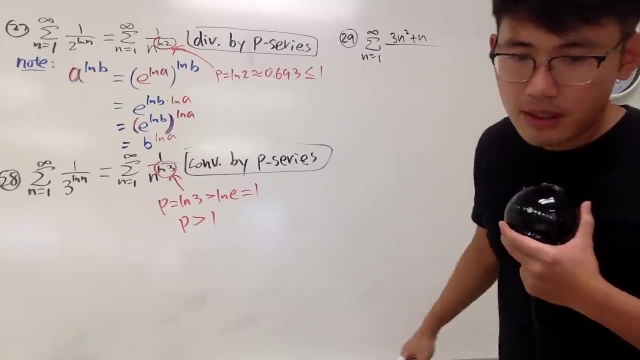 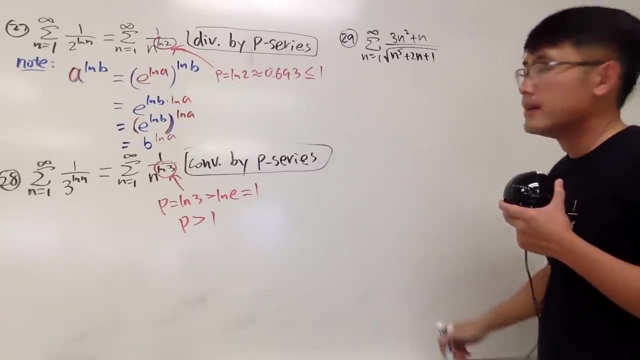 We are going to do the sum as n goes from 1 to infinity, And then we have 3n squared plus n over Square root of n to the 5th power, plus 2n plus 1, like this Okay. 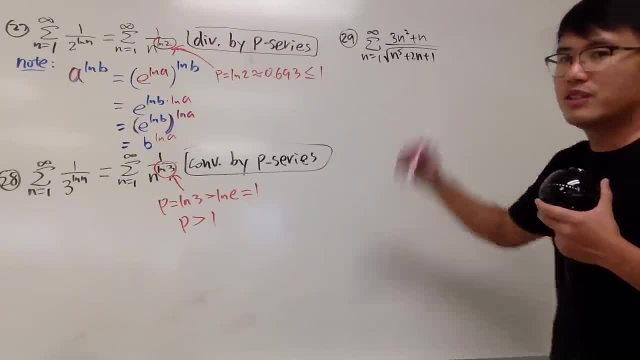 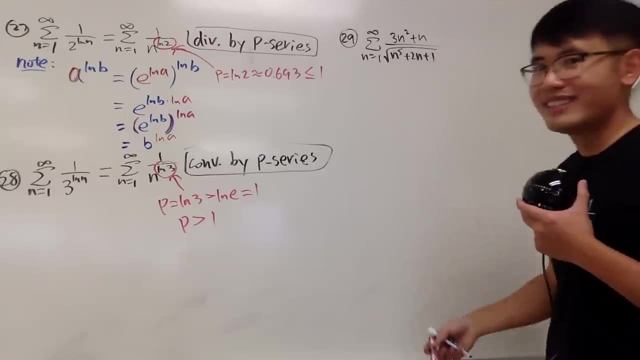 Well, it's a big rational expression and all that, So I will try to just pick the dominating part. Luckily there's no like weird natural log of whatever, So just like polynomial inside here of the square root and all that. 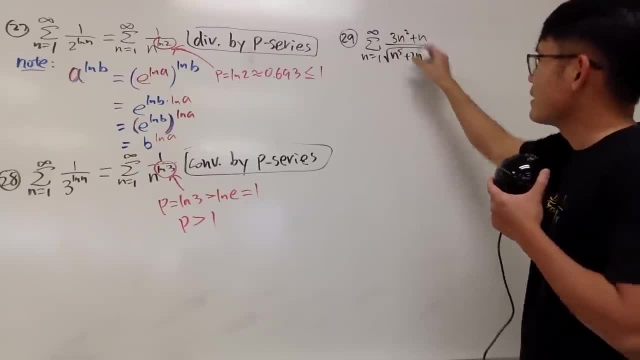 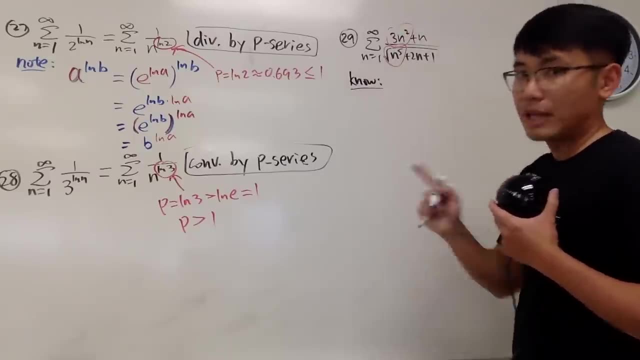 This is not polynomial because of square root, but I'm saying inside: Okay, So just look at the powers, So look at this and look at that, And perhaps, Perhaps, this is what we know much better, right? So put down what we know. 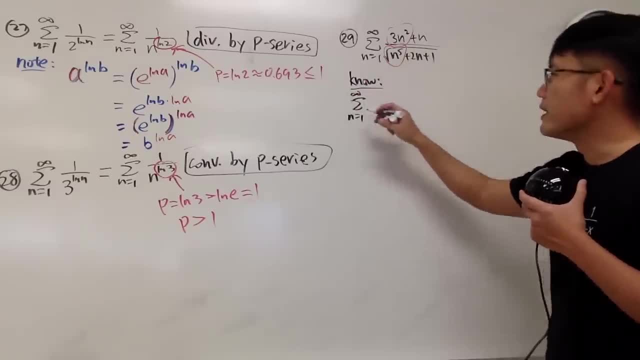 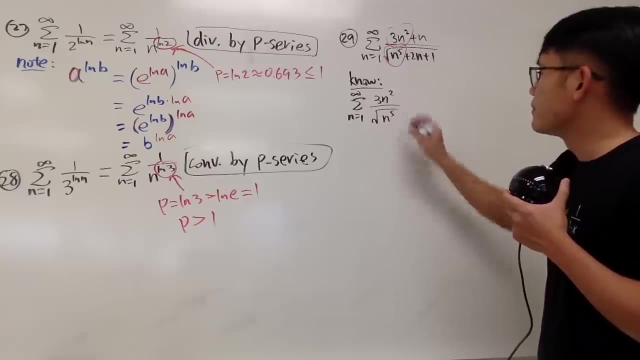 I will just write down the sum as n goes from 1 to infinity, And then here on the top we have 3n squared over square root of n to the 5th power, like this: Okay, Here's the deal. 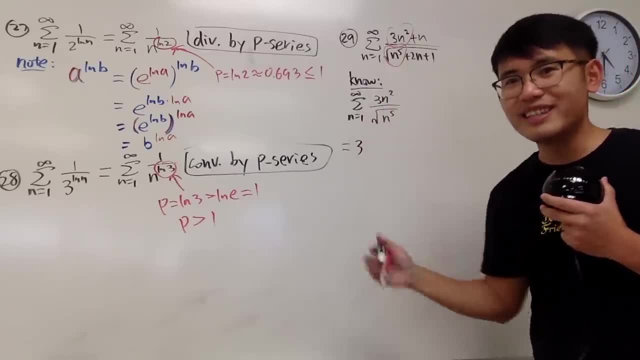 We can put the 3 in the front. This is a constant multiple. So just that integration. you can take that all the way to the front, That's okay. And then we have the sum, As n goes from 1 to infinity. 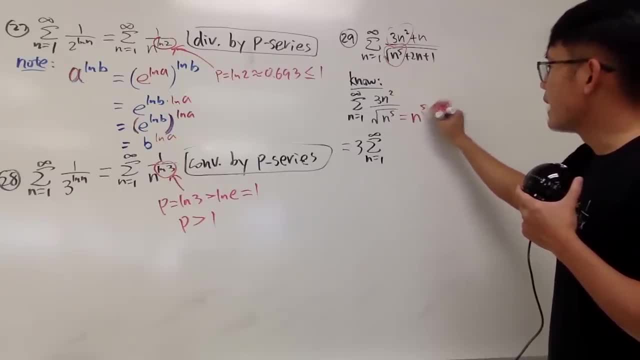 And notice this right here it's like saying n to the 5 over 2 power. Now, on the top we have 2. And on the bottom we have 5 over 2.. So in another word, this right here it's actually the same as saying: 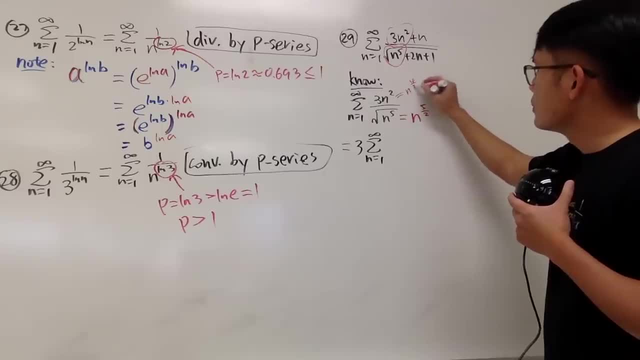 This is like saying n to the 4 over 2.. Right, So we actually have just n to the 1 half on the bottom. So all in all, I'll just put down 1 over n to the 1 half. 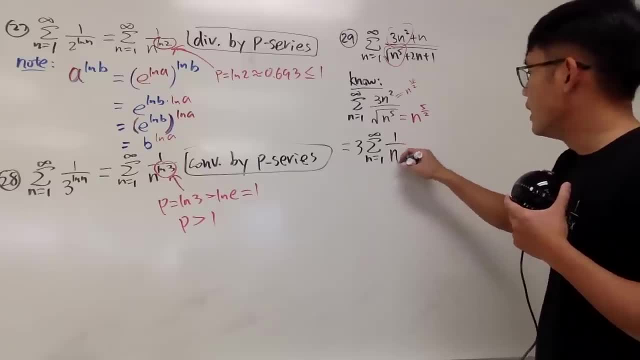 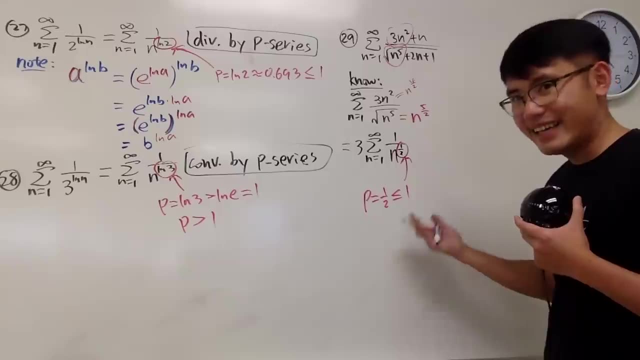 1 half on the bottom. So I'll just put down 1 over n to the 1 half and notice this right here: p is 1 half, which is less than or equal to 1, and this is a divergent. 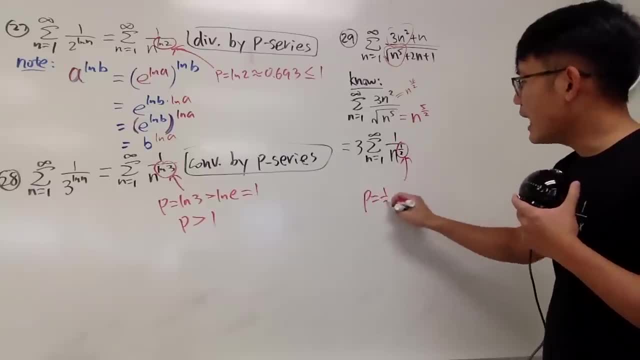 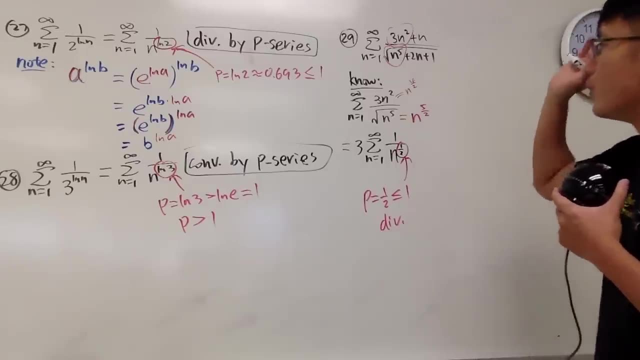 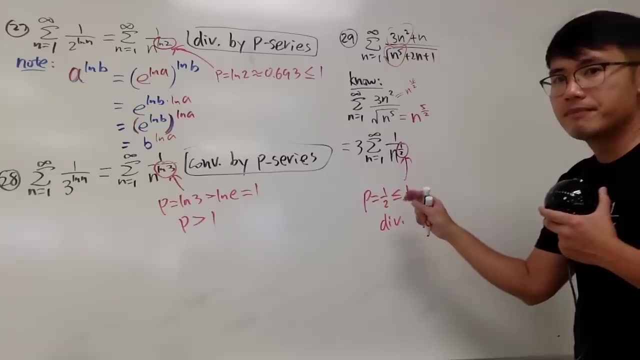 And notice this right here: p is 1 half, which is less than or equal to 1.. And this is a divergent that we know And again, we'll just pick this from here, But not done yet. We are going to compare this and that. 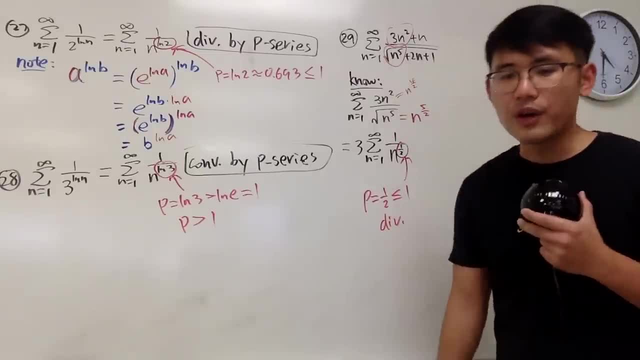 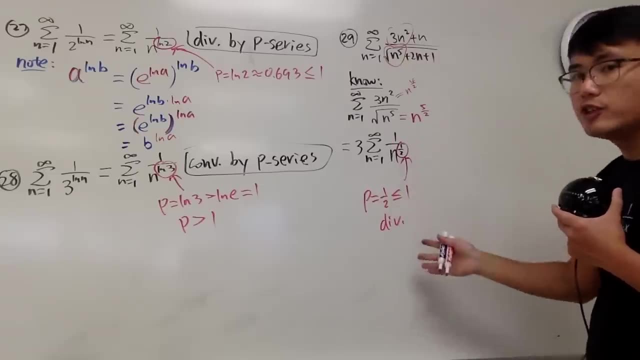 that we know And again, we just pick this from here But not done yet. We are going to compare this and that And because this is a divergent, we hope to show this right here- is bigger than the divergent right. 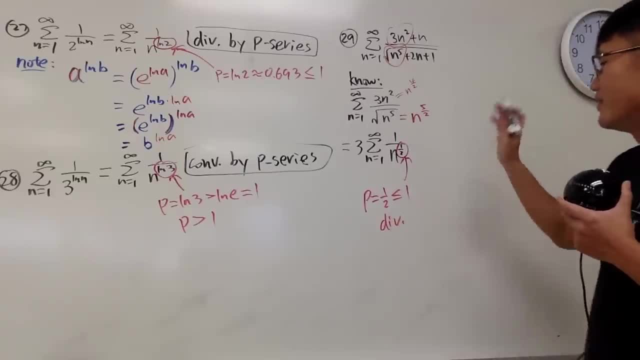 So, in another word, it's like if you have, like if you. if you don't like to use an old or older analogy, you can use like if you are rich, if you are richer than a rich person, you are rich. 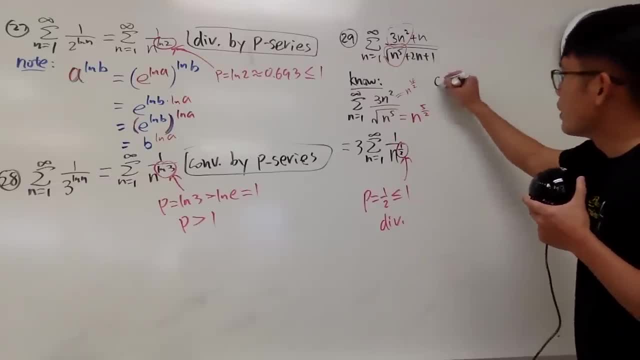 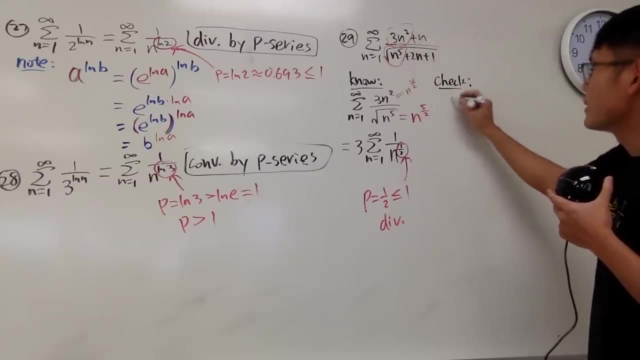 as well, more rich, much better. Anyway, here we go. This is the check. We are going to just seriously check the inside, okay, So you just check. still put down: the sum n goes from 1 to infinity. 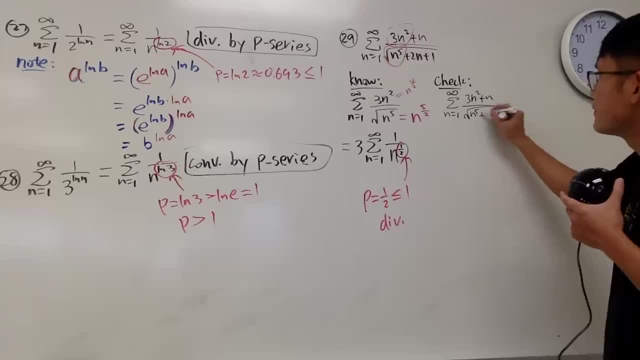 3n squared plus n over square root of n. fifth plus 2n plus 1.. I want to check if this series is bigger than or equal to. I don't know yet, so I'll put down a question mark Then that. 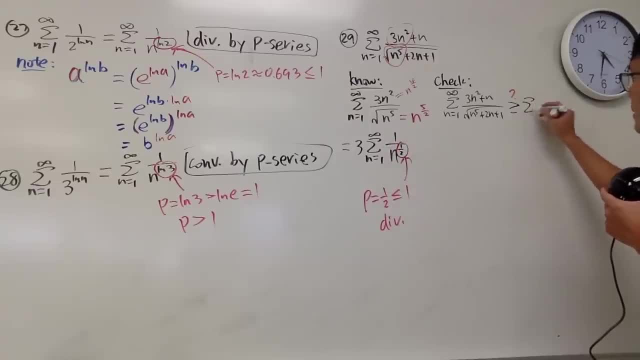 And I will keep the 3 as well. So the sum as n goes from 1 to infinity is 3,. okay, over n let's put down square root, why not? And here we just care about, for n is greater than or equal to 1.. 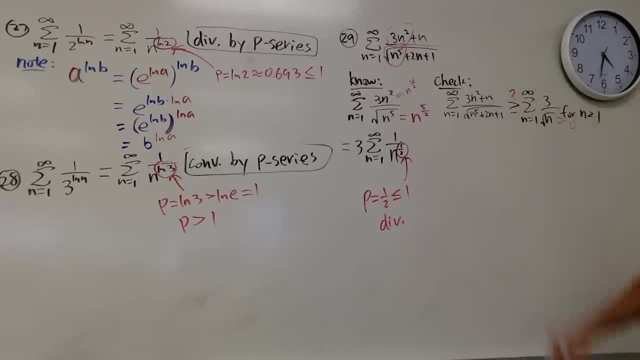 And again you should also indicate that this right here is positive. everybody is positive here. that's nice. Take out this series right, just the expression 3n squared plus n over square root of n to the fifth power and. 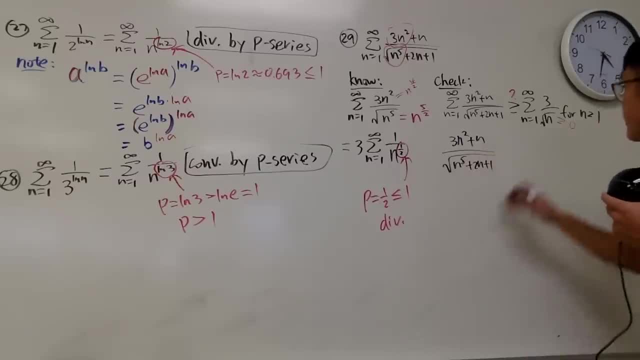 we add 2n plus 1, and we will check if this is greater than or equal to 3 over square root of n. And you see, this is much harder if you just talk about, like you know, take out something and all that. so that's why it might be. 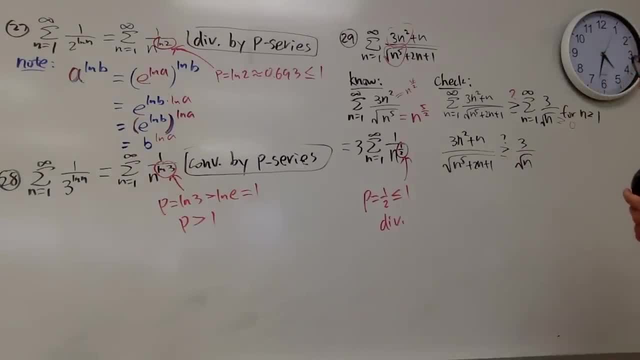 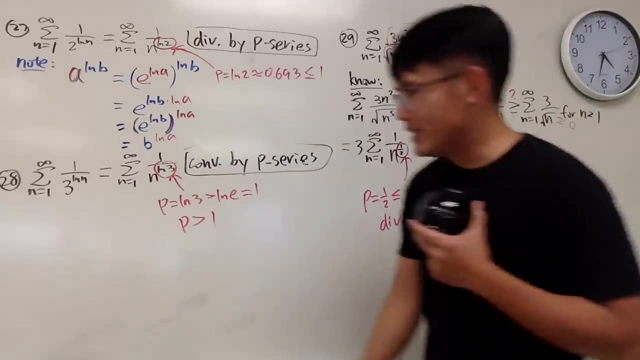 a better idea to just do this? Or why don't we just do the? why don't we just do a limit? huh, Maybe limit is even better. Yeah, and let's actually, let's- try to do a limit, because this is a lot of algebra to do, it's not? 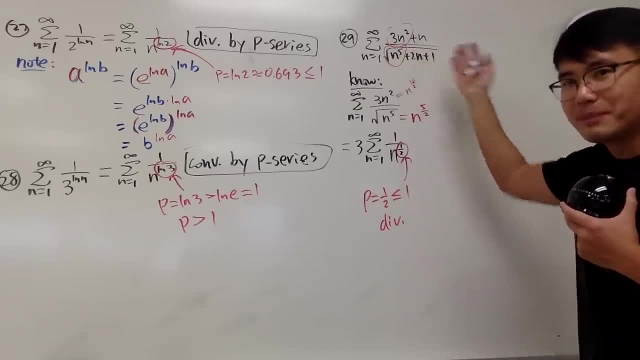 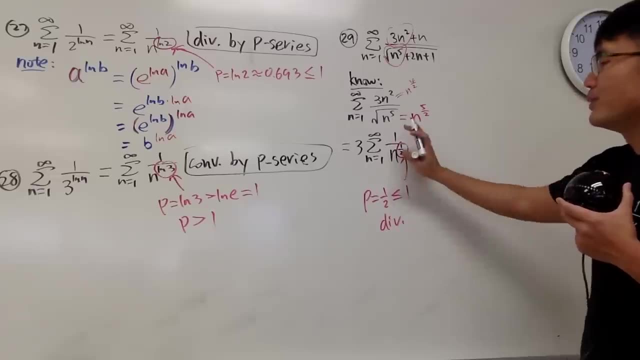 And because this is a divergent, we hope to show this right here- It's bigger than the divergent right. So, in other words, like if you have, like If you, If you don't like to use an old or older analogy, you can use like if you are rich. 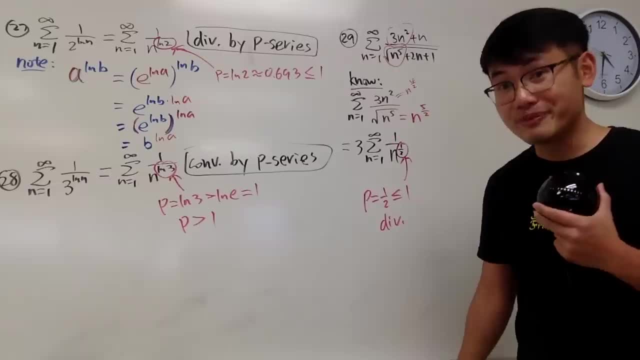 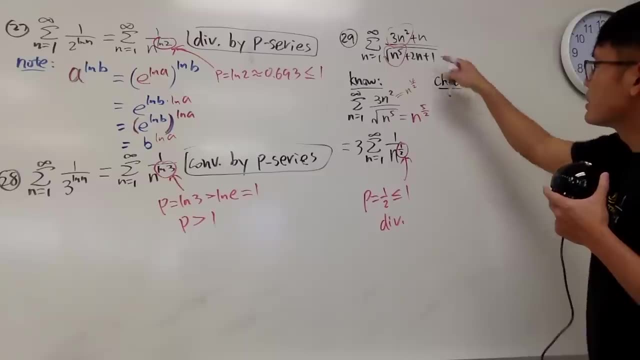 If you are richer than a rich person, you are rich as well, More rich, Much better. Anyway, here we go. This is the check. We are going to just seriously check the inside. okay, So you just check. Still, put on some. 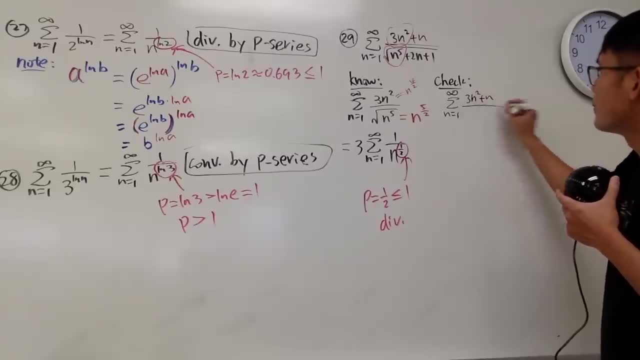 n goes from 1 to infinity: 3n squared plus n over square root of n. fifth plus 2n plus 1.. I want to check if this series is bigger than or equal to. I don't know yet, so I'll put down a question mark. 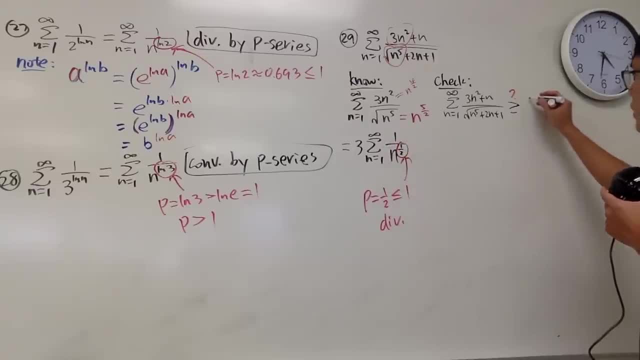 Then that, And I will keep the 3 as well. So the sum as n goes from 1 to infinity 3, okay, over n Let's put down square root, Why not? And here we just care about, for n is greater than or equal to 1.. 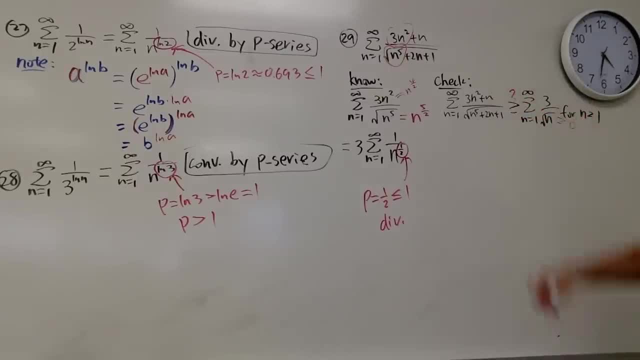 And again you should also indicate that this right here is positive. Everybody is positive here. That's nice. Take out this series, right, Just the expression 3n squared plus n over square root of n to the fifth power, And we add 2n plus 1.. 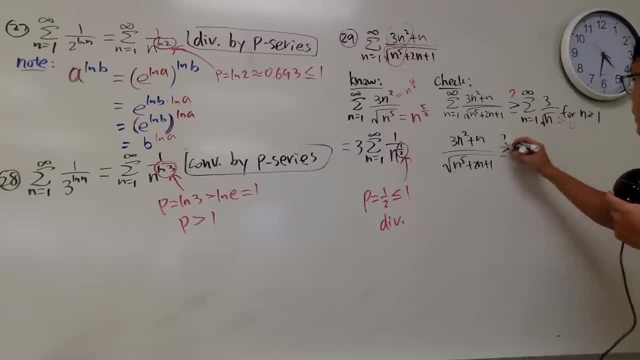 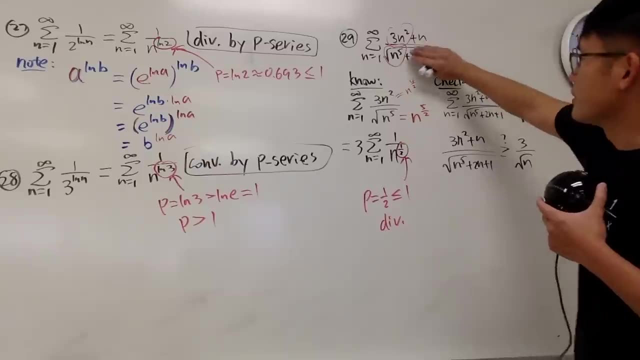 And we will check if this is greater than or equal to 3 over square root of n. And you see, this is much harder if you just talk about, like you know, take out something and all that. So that's why it might be a better idea to just do this. 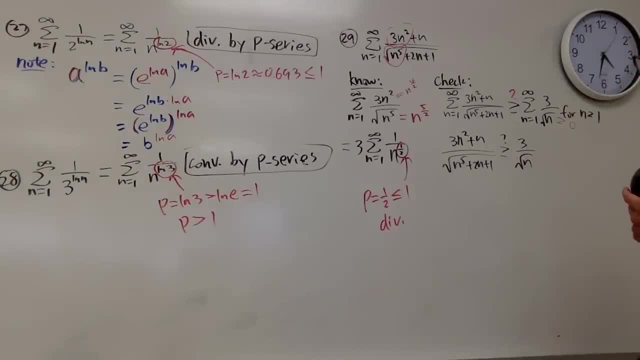 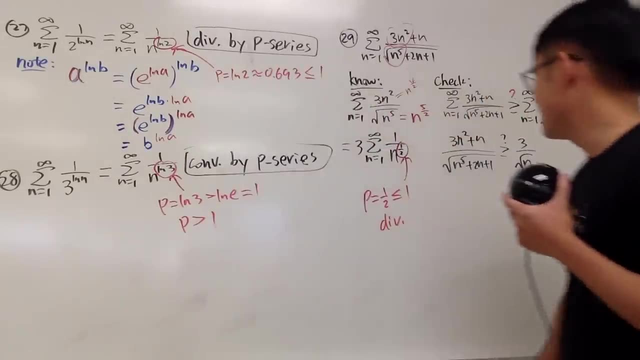 Or why don't we just do the? Why don't we just do a limit? huh, Maybe limit is even better. Yeah, and let's- actually Let's- try to do a limit, because this is a lot of algebra to do. 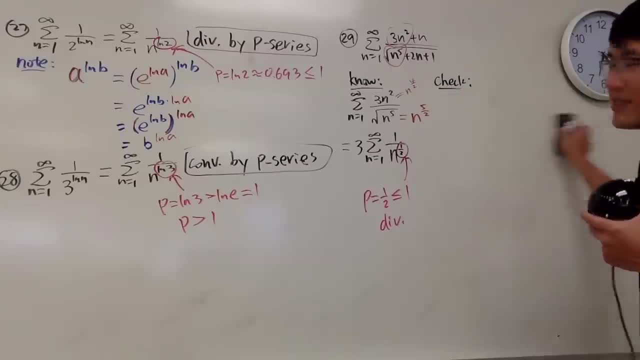 It's not fun at all. So let's actually try to do a limit comparison test. Maybe it works as well. You should, Anyway. so to check, let's do a limit comparison test On the top. I will just do 3n squared plus n over square root of n to the 5 plus 2n plus 1. 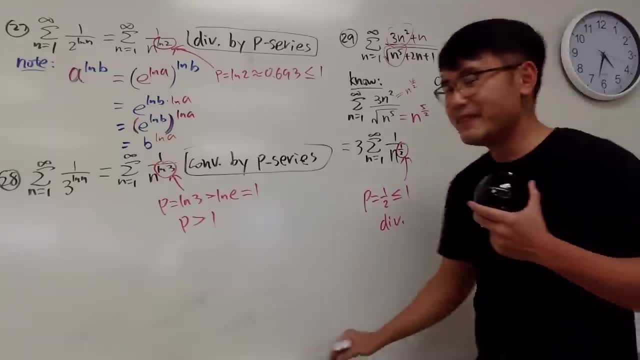 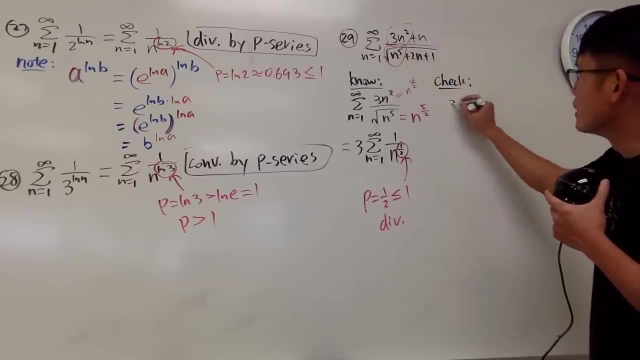 fun at all. So let's actually try to do a limit comparison test. Maybe it works as well, Anyway. so to check, let's do a limit comparison test On the top. I will just do 3n squared plus. 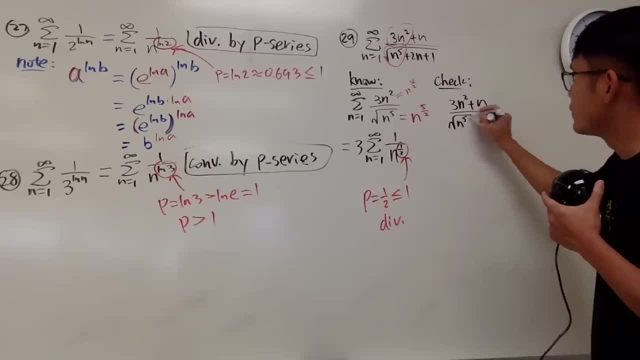 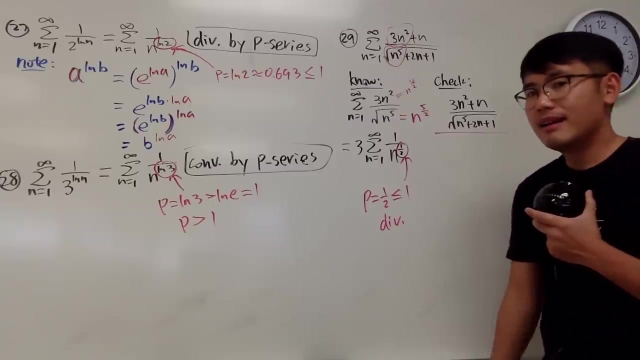 n over square root of n to the 5 plus 2n plus 1, divided by the one that we know much better. You can put this down or you can put down the 3,. seriously, it's up to you. Let me just. 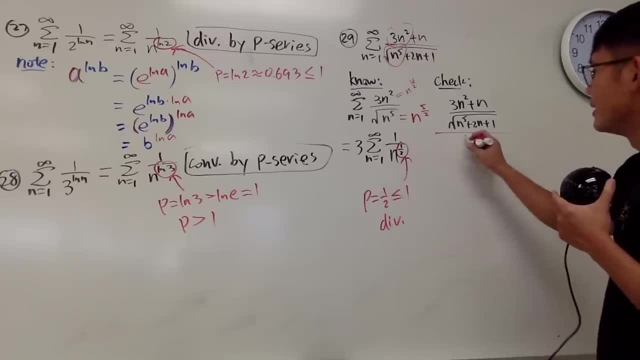 put down the seriously up to you. I'll just put down 3, not to cause any confusion. so I'll just put down 3 over, so to put the 3 right here, back right outside here, And then you have n to. 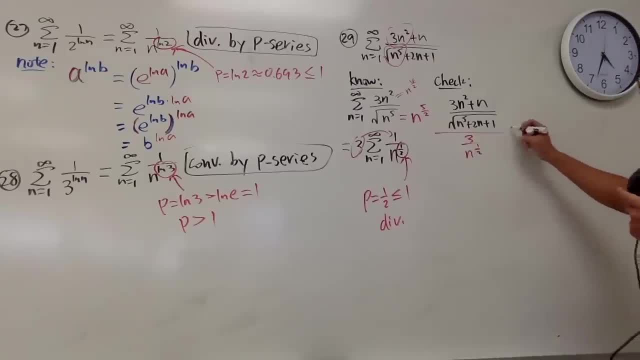 the one-half power. Now do some algebra This right here on the top. you get 3n squared plus n over square root of n, 5 plus 2n plus 1.. And you multiply by this is n to the one-half. 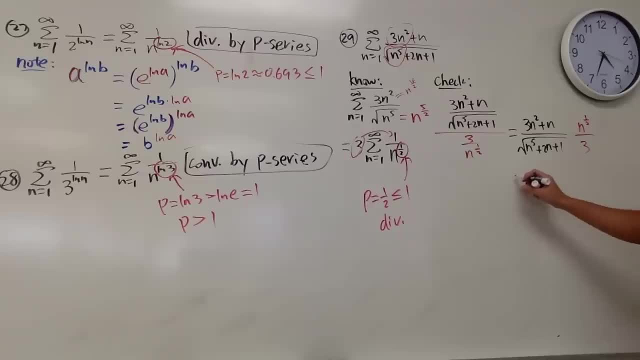 divided by 3.. And now here is the deal. Let me just put this down right here. Well, take this: multiply, multiply, right. So on the top we get 3n, this times that we get 5 over 2, and then this is: 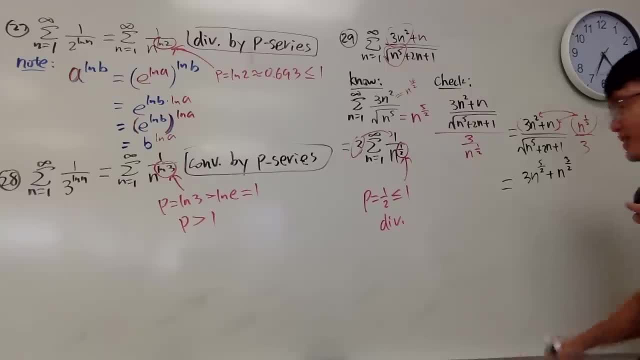 plus n to this 3 over 2 after you multiply the powers. Well, after you multiply and you add the powers, and then right here you have 3 in front of the square root and 5 plus 2n plus 1.. 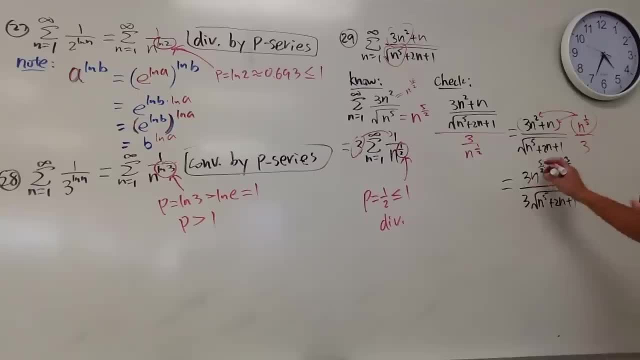 Now pick the dominating part for the power situation, right, Pick this and pick that And you see this right here is actually the same as this. So you can conclude that this right here actually just go to 1.. So they are. 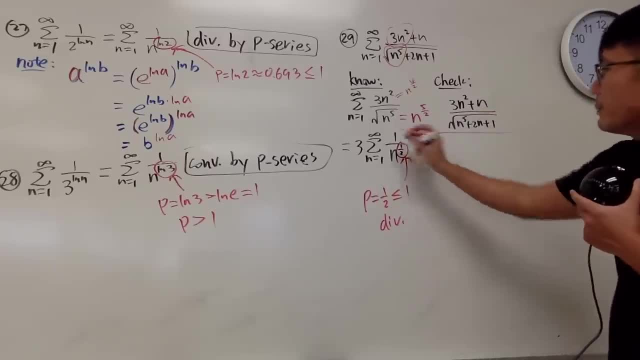 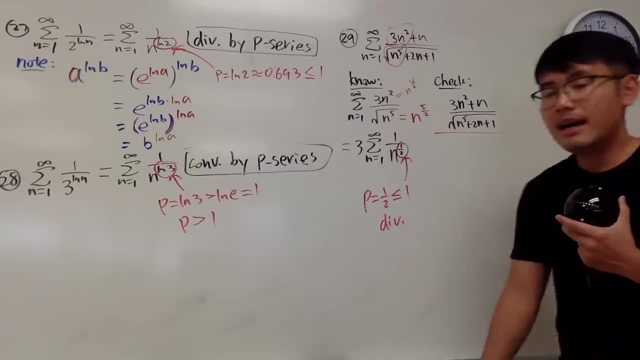 divided by the one that we know much better. You can put this down. You can put this down or you can put down the 3.. Seriously, it's up to you. Let me just put down the. Seriously, it's up to you. 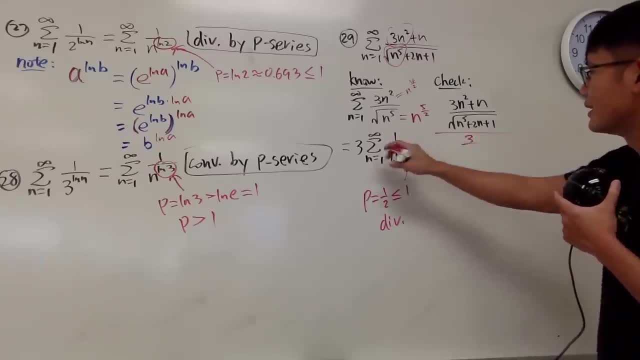 I'll just put down the 3, not to cause any confusion. So I'll just put down 3 over. So just put the 3 right here, back, right outside here, And then you have n to the 1 half power. 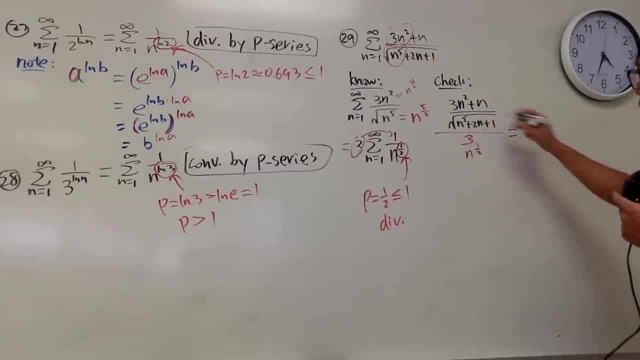 Now do some algebra This right here on the top you get 3n squared plus n over square root of n to the 1 half plus n over square root of n to the 5 plus 2n plus 1.. 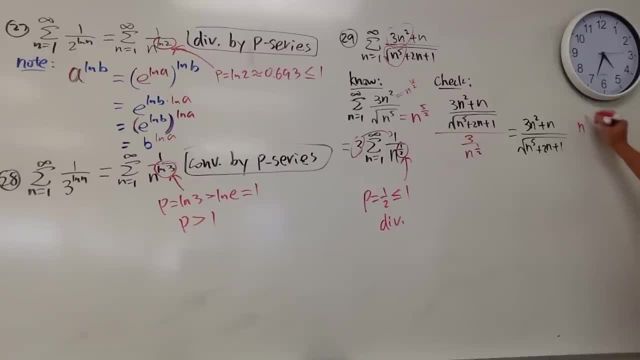 And you multiply by. This is n to the 1 half divided by 3.. And now here is the deal. Let me just put this down right here. Well, take this: multiply, multiply, right. So on the top we get 3n. 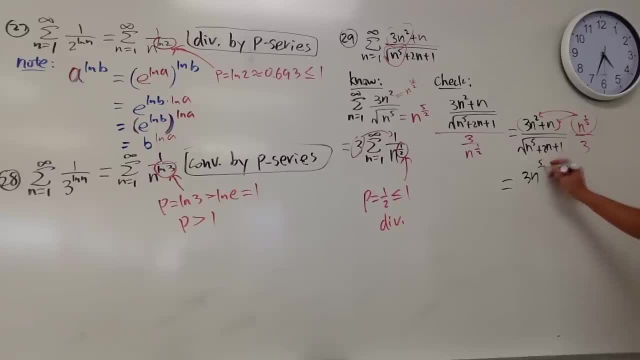 This times that we get 5 over 2.. And then this is plus n to the 3 over 2 after you multiply the powers. Well, after you multiply and you add the powers, And then right here, you have 3 in front of the square root. 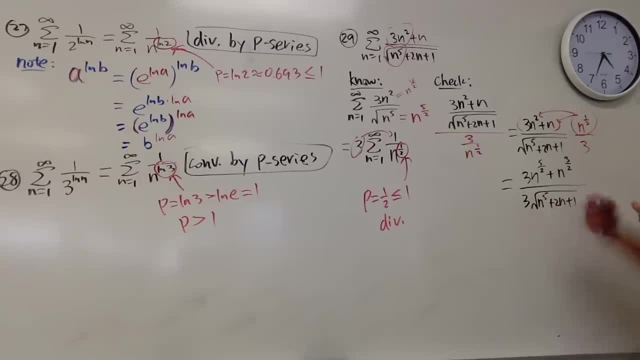 And 5 plus 2n plus 1.. Now take the dominating part For the power situation, right, Take this and take that And you see this right here is actually the same as this, So you can conclude that this right here actually just go to 1.. 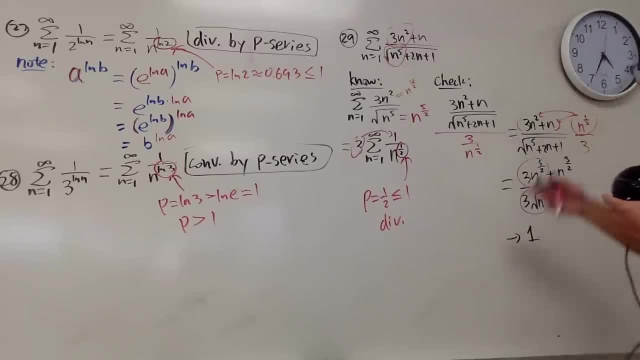 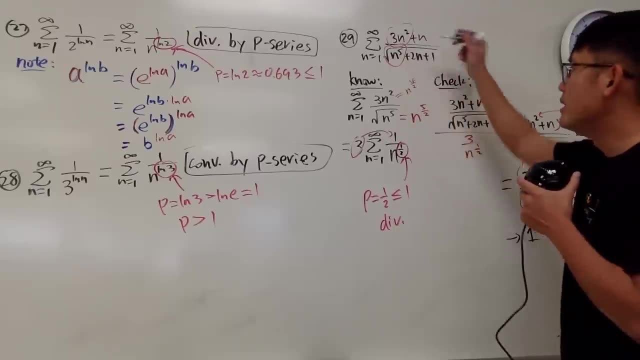 So they are pretty much of the same size, right? So that's pretty much the work you can do. So this is 1, which is greater than 0. We can draw a conclusion, Come back here and say this right here: 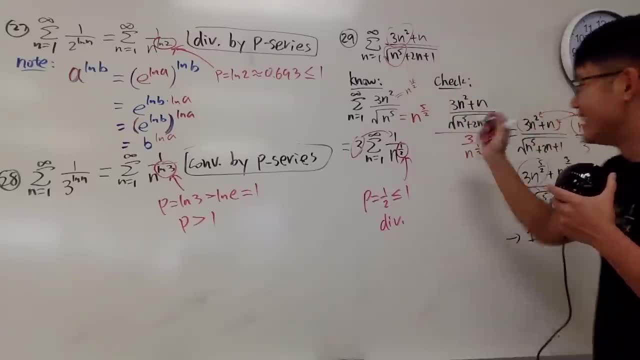 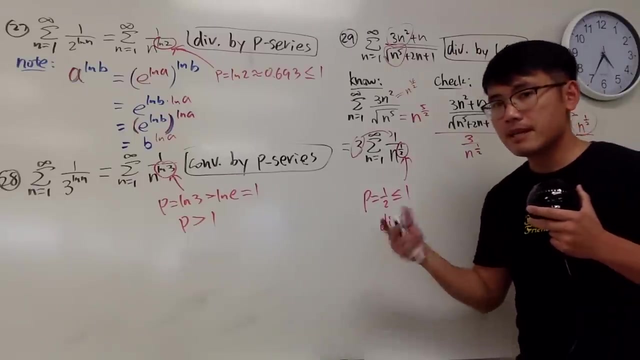 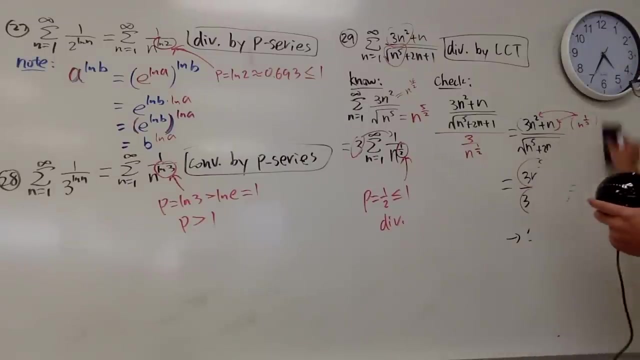 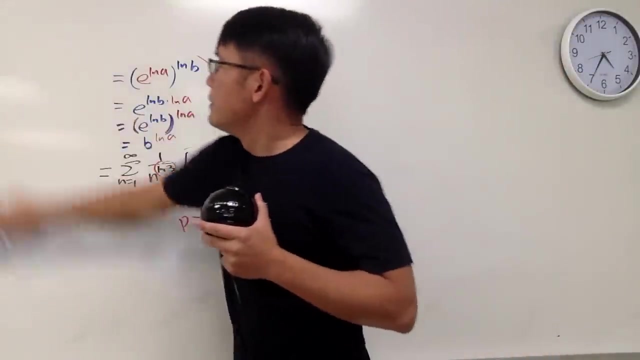 Well, sorry, Also diverges. This right here also diverges Because of the limit comparison test. I think it's much easier to do limits than Inequality from algebra. So this is it right, Number 29. So save energy. 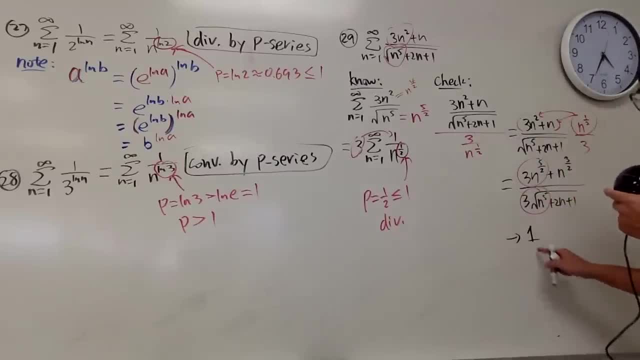 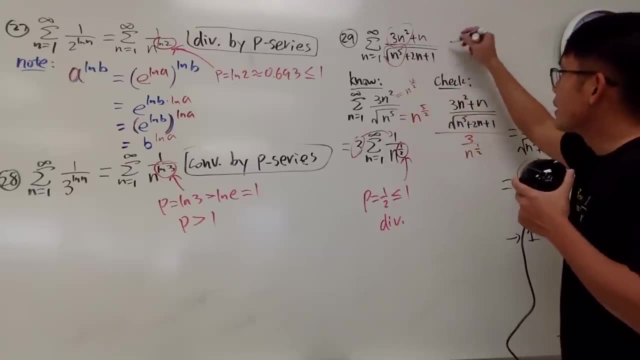 pretty much of the same size, right? So that's pretty much the work you can do. So this is 1,, which is greater than 0. We can draw a conclusion. Come back here and say this right here: well, sorry, also diverges. 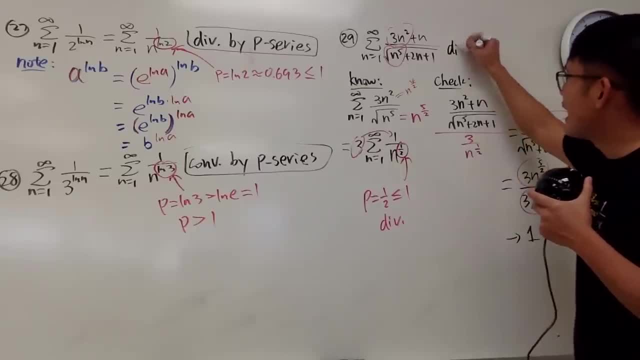 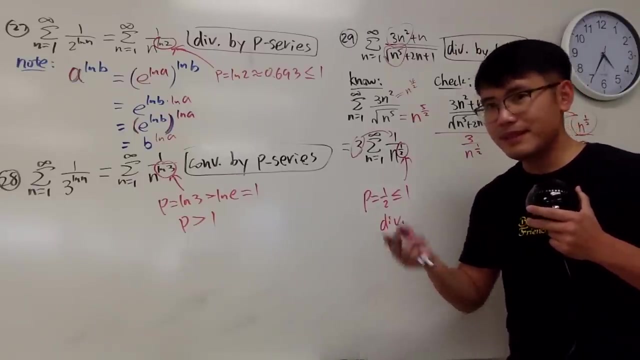 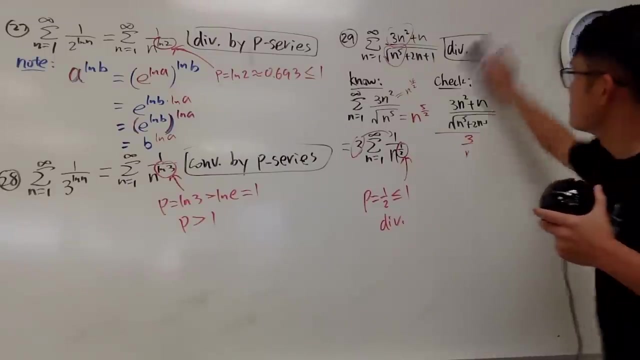 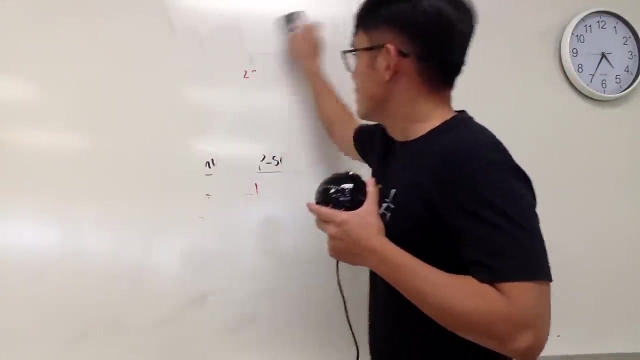 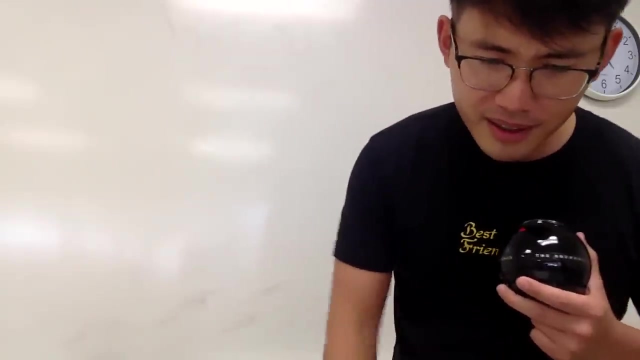 This right here also diverges Because of the limit, computer syntax. I think it's much easier to do limits than inequality from algebra. So this is it, alright, Number 29.. So save energy, Okay, anyway, Number 30.. 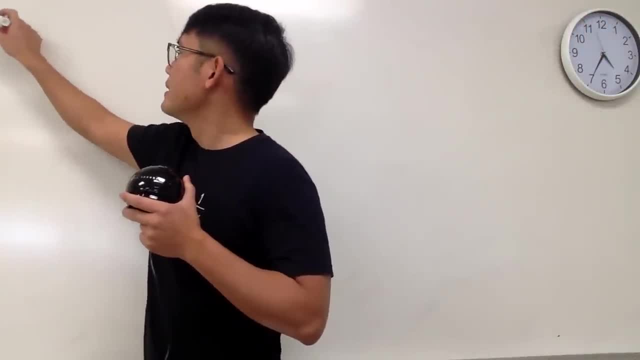 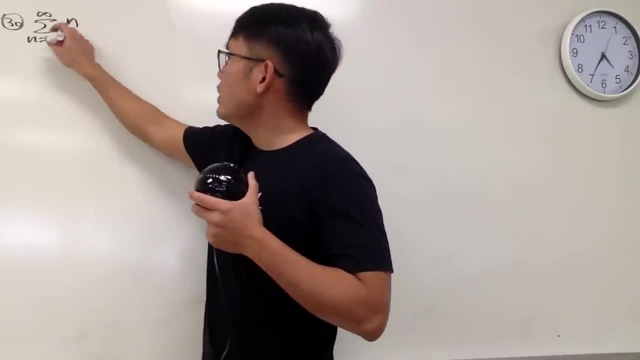 We are going to calculate this guy, Number 30,, right, Number 30. We are going to calculate the sum as n goes from 1 to infinity, And then we have n over 2.. Are you serious? This is not geometric series. 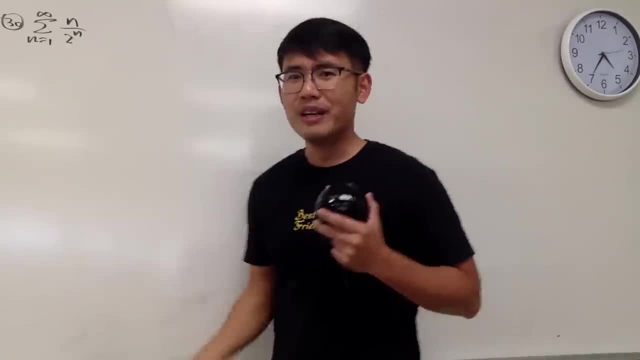 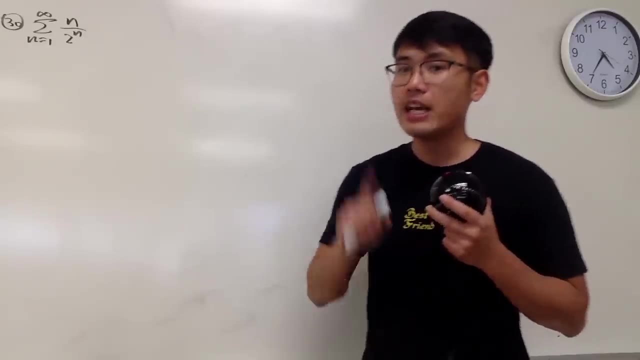 that I know. Put the n right here. Give me back my 1.. Don't worry, We can still do this nicely. Here is the deal. Let me show you. So let me just write down the expanded version for you guys. 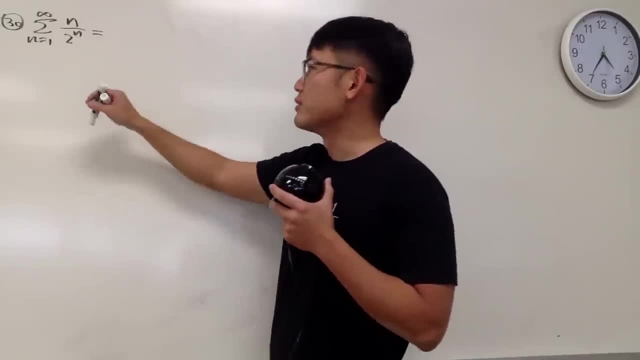 real quick If you put down 1,, 2,, 3,, 4,, 5, and to the n's right. So let me just write down a few of them for you guys. So when you do that, you get 1 over. 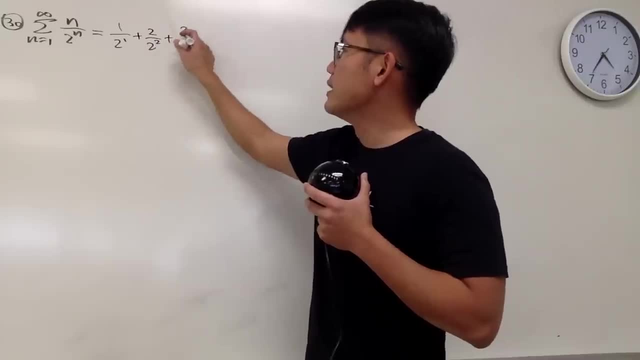 2 to the first power, plus 2 over 2 to the second, plus 3 over 2 to the third, plus 4 over 2 to the fourth, and then so on, so on, so on. right And now. 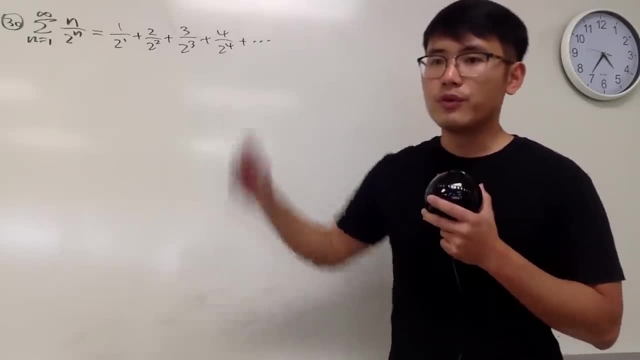 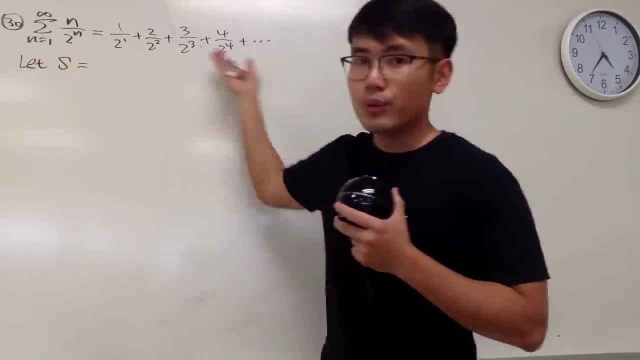 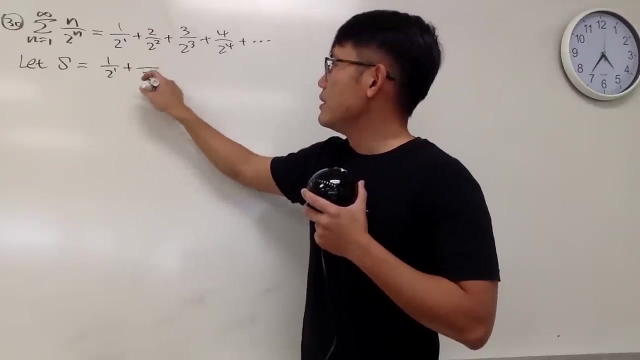 this is the usual approach that we do for this kind of sum. First of all, we can say that s for the sum okay, Equal to this expression, which is 1 over 2 to the first, plus 2 over 2 to the second. 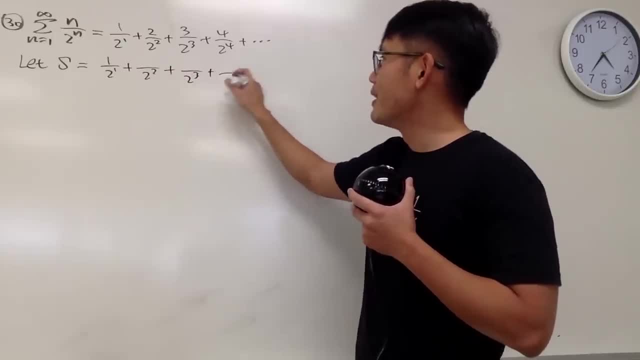 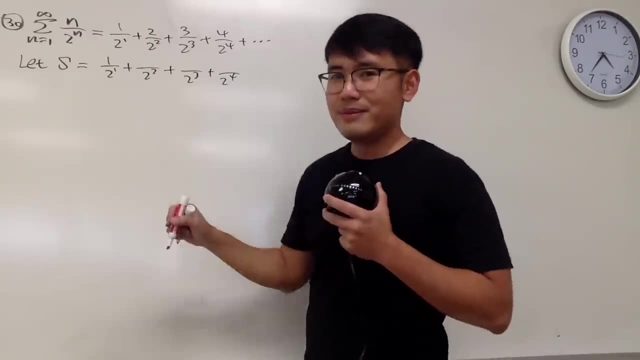 plus 3 over 2 to the third, plus 4 over 2 to the fourth, and so on, which is just this. We call that to be the sum. And now check this out: 1,. I mean everybody. 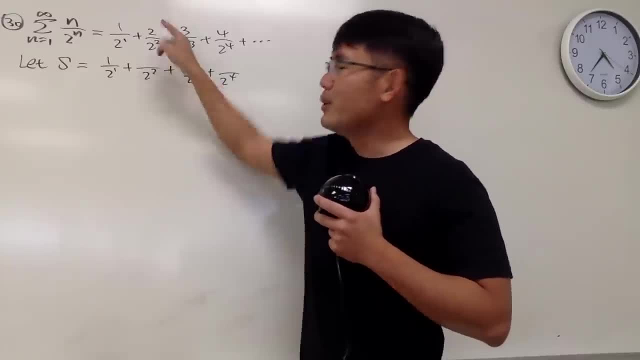 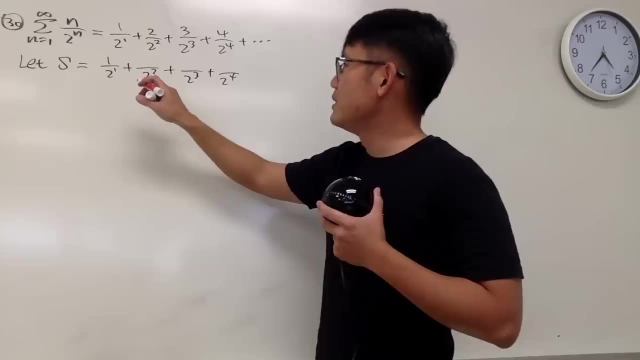 knows 1 plus 1 is equal to 2.. But I know 2 is the same as 1 plus 1.. I almost forget about my jokes. But anyway, this right here. let me see what color should I put this down? 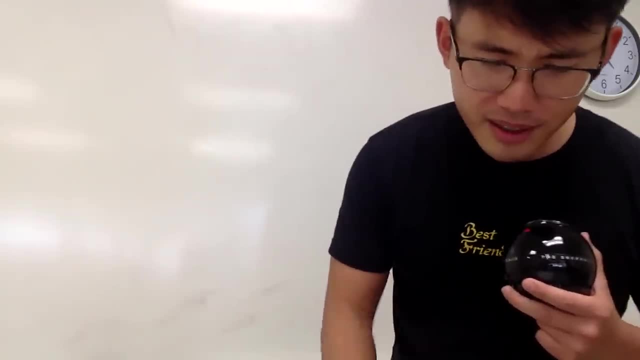 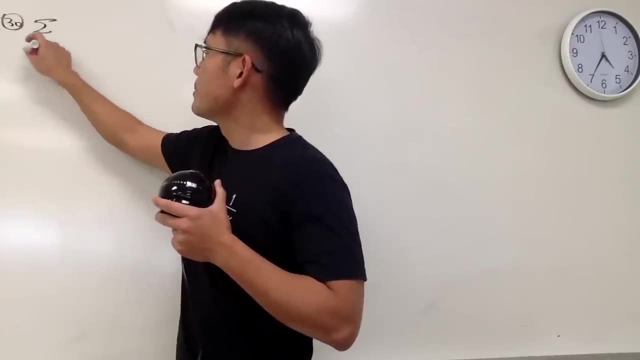 Okay, anyway, Number 30.. We are going to calculate this guy, Number 30,, right, Number 30.. We are going to calculate the sum as n goes from 1 to infinity, And then we have n over 2.. 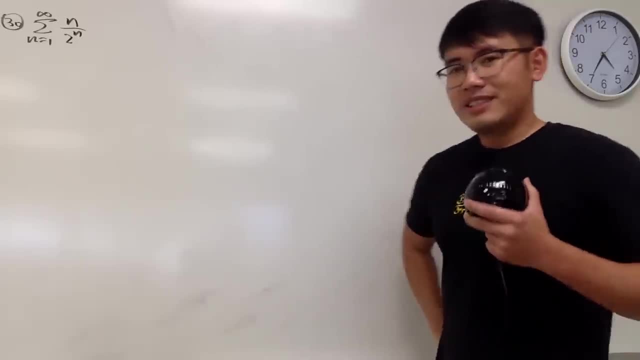 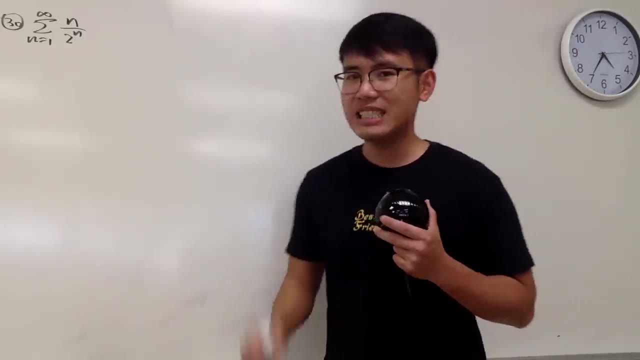 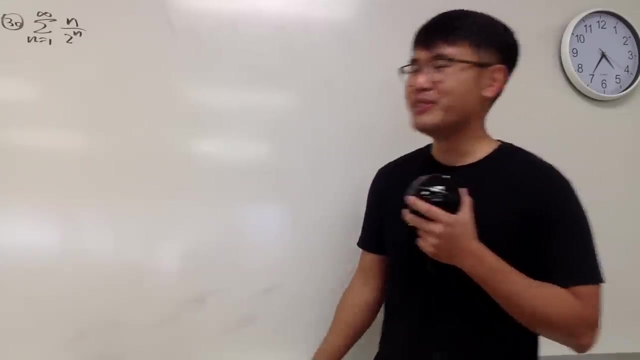 Are you serious? This is not a geometry series that I know. We put the n right here. Give me back my 1.. God Don't worry, We can still do this nicely. Here is the deal. Let me show you. 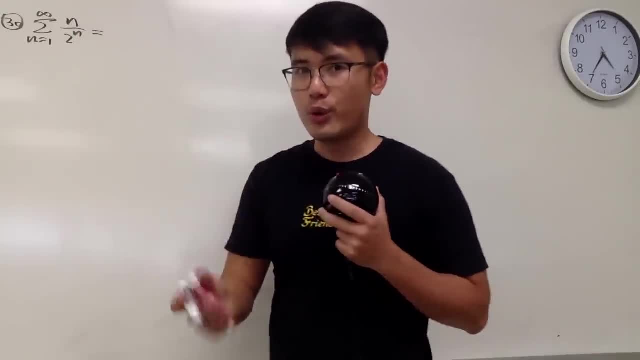 So let me just write down the expanded version for you guys real quick, If you put down 1,, 2,, 3,, 4,, 5, and to the n's right. So let me just write down a few of them for you guys. 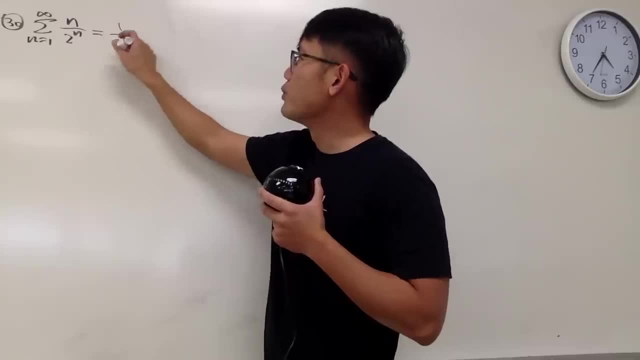 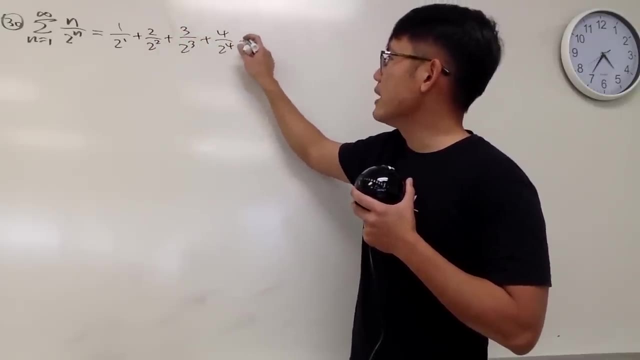 So when you do that, you get 1 over 2 to the first power, plus 2 over 2 to the second, plus 3 over 2 to the third, plus 4 over 2 to the fourth, and then so on, so on, so on, right. 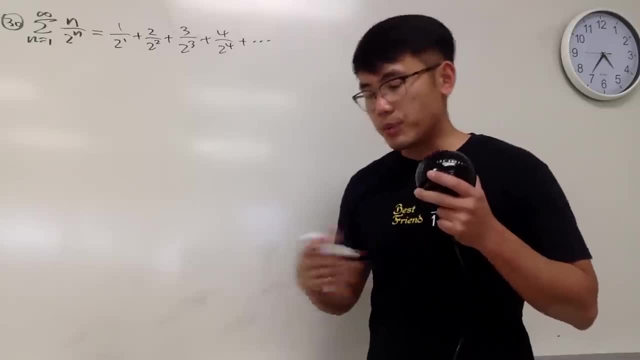 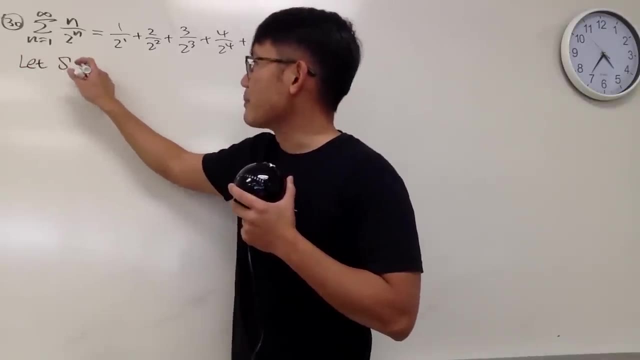 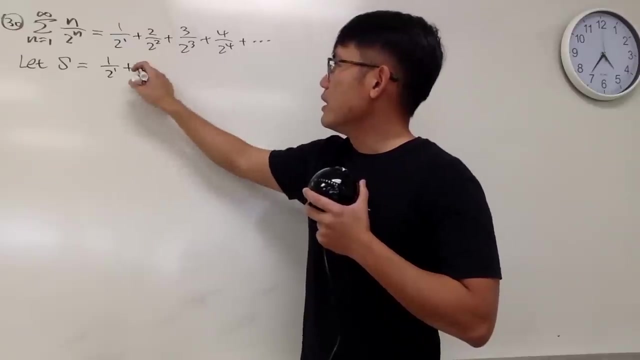 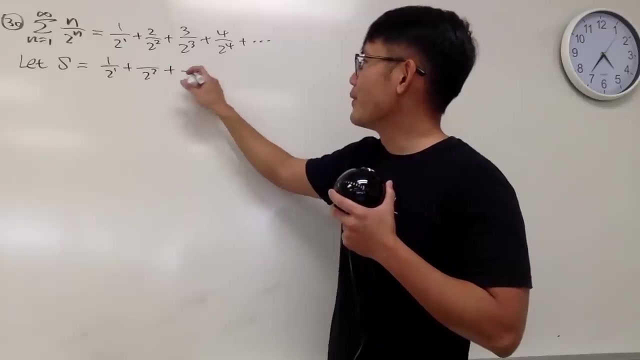 And now, this is the usual approach that we do for this kind of sum. First of all, we can say that s for the sum, okay, Equal to this expression, which is 1 over 2 to the first, plus 2 over 2 to the second, plus 3 over 2 to the third, plus 4 over 2 to the fourth, and so on, which is just this. 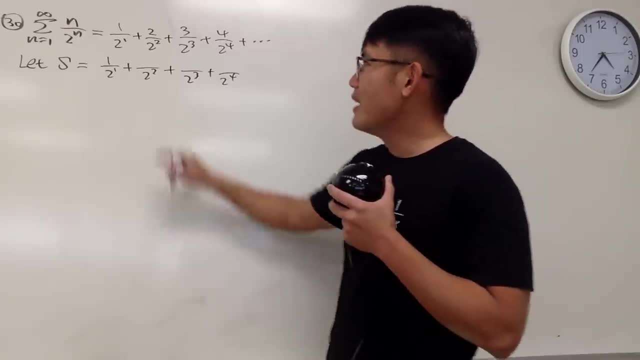 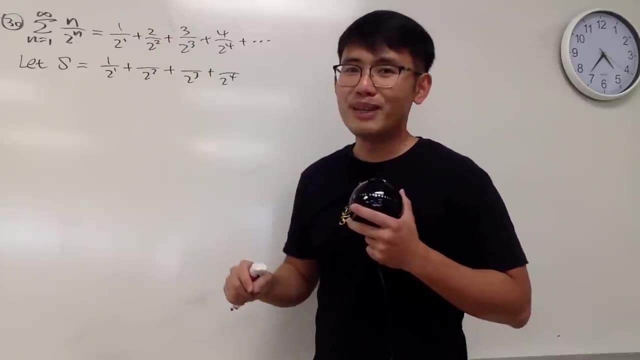 We call that to be the sum. And now check this out: 1, I mean, everybody knows 1 plus 1 is equal to 2.. But I know 2 is the same as 1 plus 1.. I almost forget about my jokes. 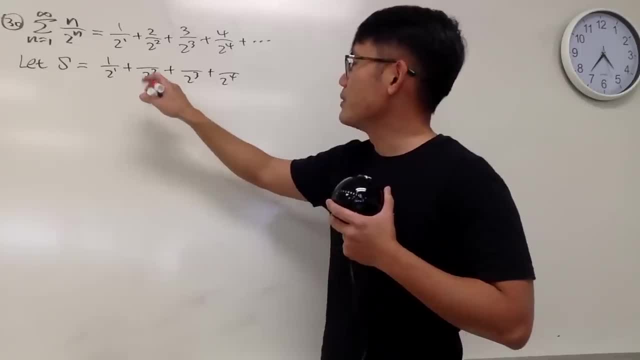 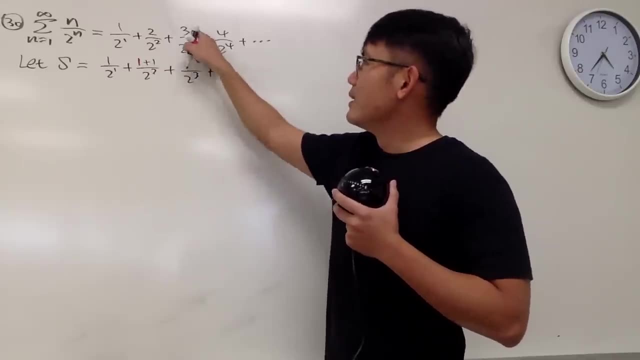 But anyway, this right here. Let me see What color should I put this down. So I just put down 1 in red plus 1 in black. Let's look at 3.. 3 is the same as 1 plus 2.. 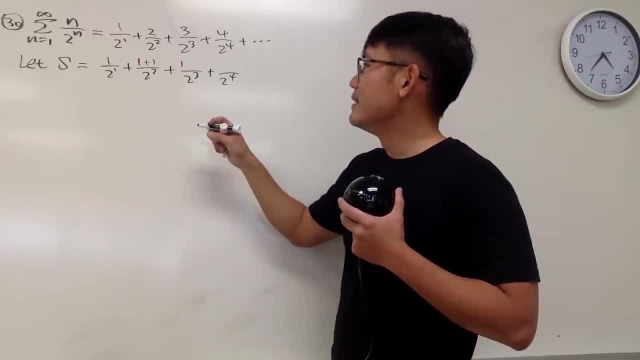 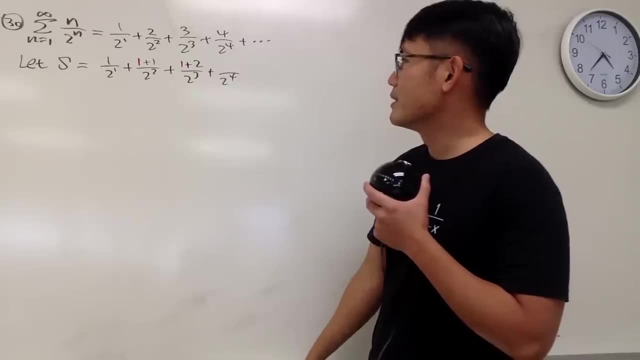 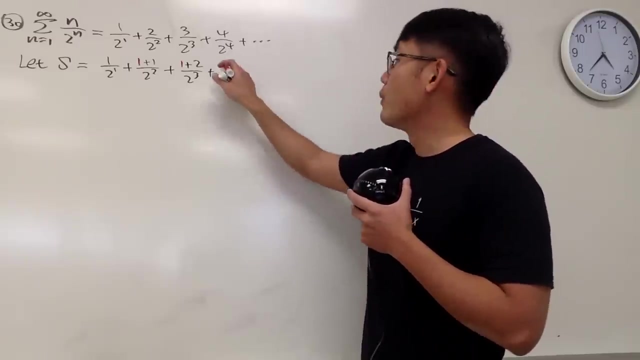 So I put down 1 in red and 2 in black, like this. I'm just thinking about what color should I do? Okay, okay, I think that should be okay. And the next is 4.. Of course, it's the same as 1 plus 3.. 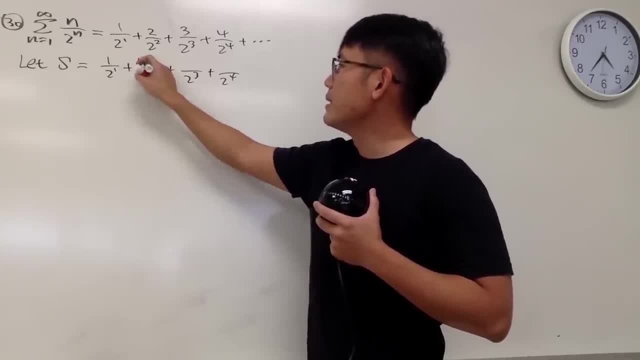 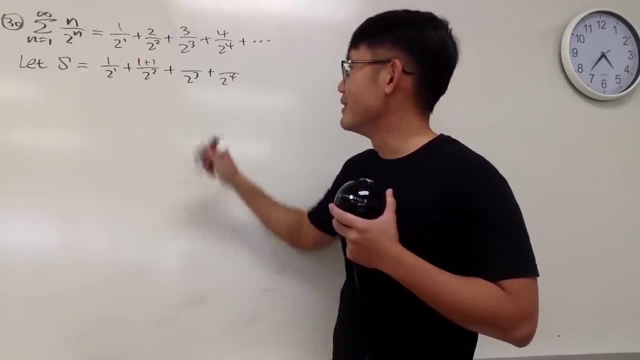 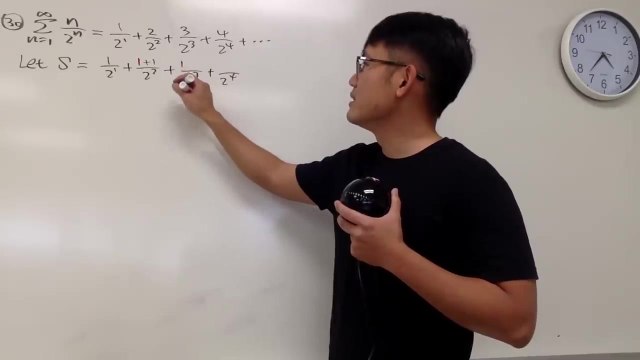 So I just put down 1 in red plus 1 in black. Let's look at 3.. 3 is the same as 1 plus 2. So I put down 1 in red and 2 in black, Like this. 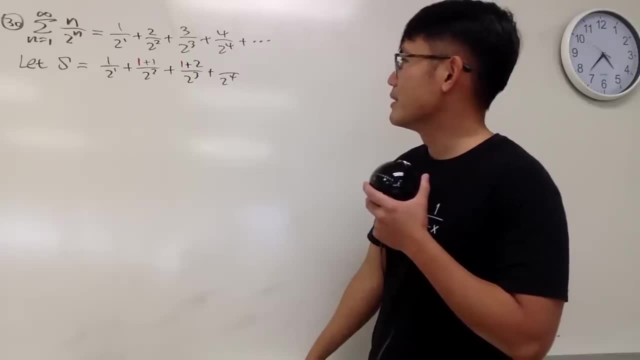 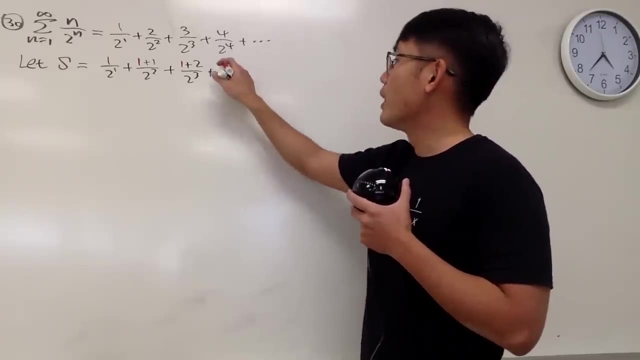 I'm just kind of thinking about what color should I do? Um, okay, okay, I think that should be okay. And the next is 4.. Of course, it's the same as 1 plus 3.. Of course, people will say: 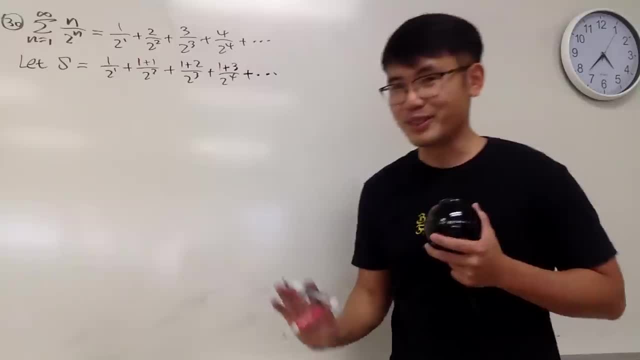 why don't you do 1 plus 1 plus 1 plus 1? No, Just don't. Alright, Now we are going to play around with this. As you can see this right here s will be the same. 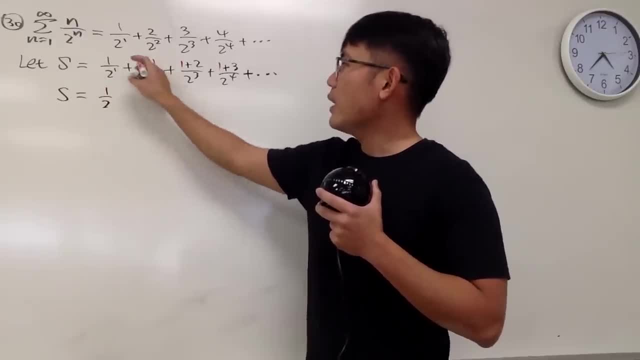 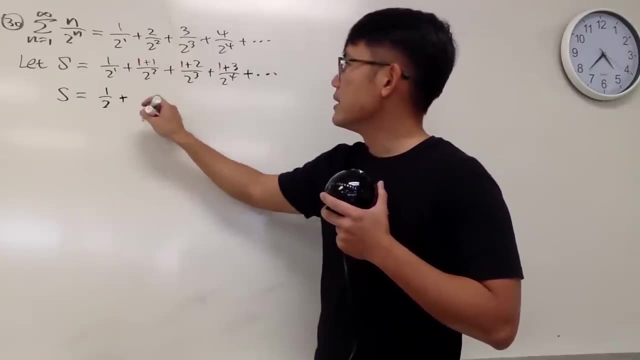 as this is just 1 half, just leave it. And now I will just leave this part in a second I will put this down right here. Plus 1 over 1 half- I'll just put everything in red. So 1 half plus. 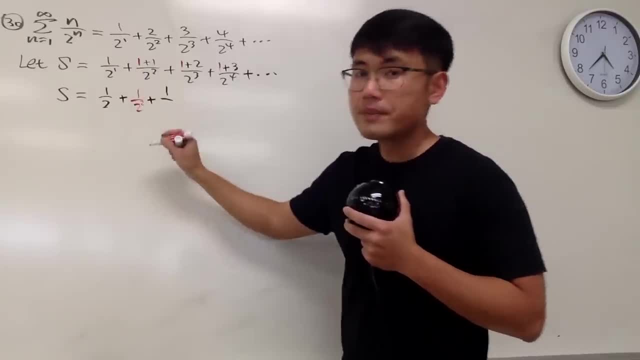 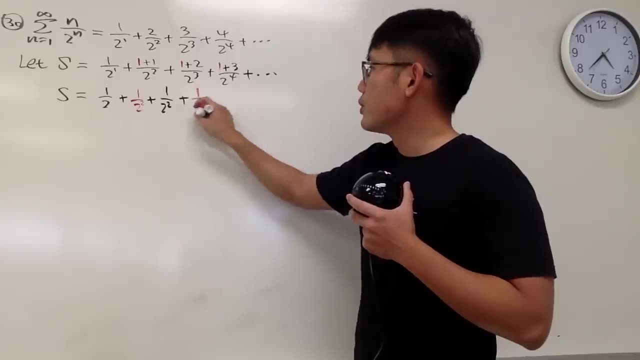 this is 1 over 2 square, And then 1 over 2 square, again black, and then this right here: plus 1 over 2 to the third power, And then this right here is plus 2 over 2 to the third power. 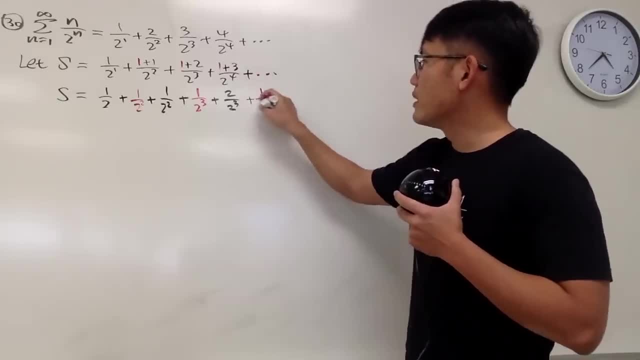 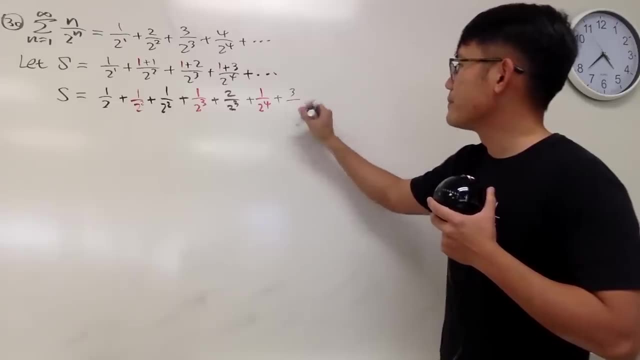 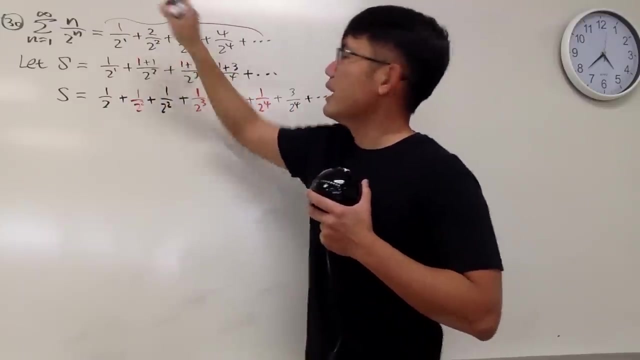 And then this right here is plus 1 over 2 to the 4th power. And then this right here is plus 3 over 2 to the and, of course, plus dot dot dot. and remember the whole thing: right here was our S right. 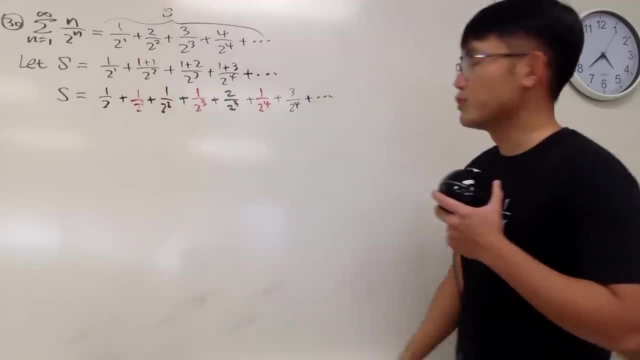 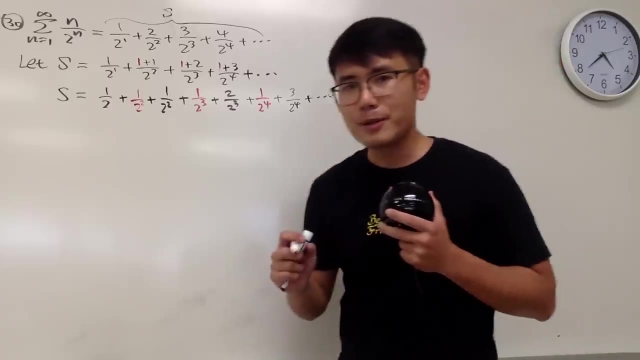 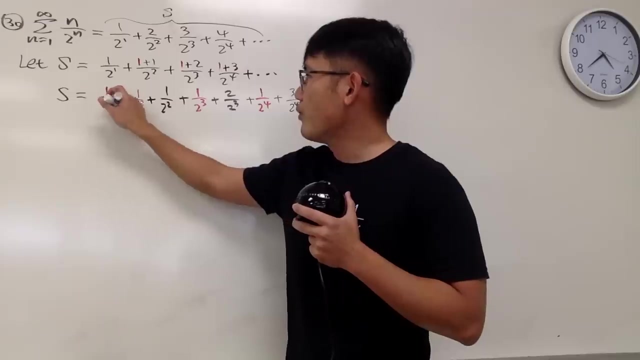 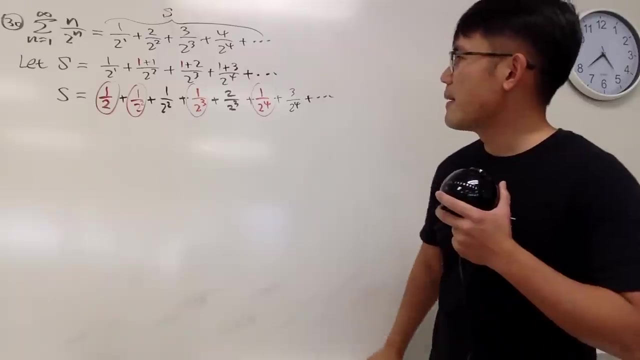 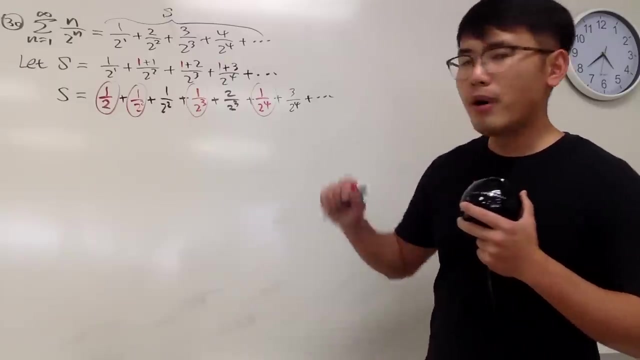 Superman. all right, check this out. hmm, check this out. check this out. check this out, okay. okay, I know how to handle this. 1 over 2. this is like this. nothing looks good to me. the red parts are just the, you know, deform the geometry series, and let's. 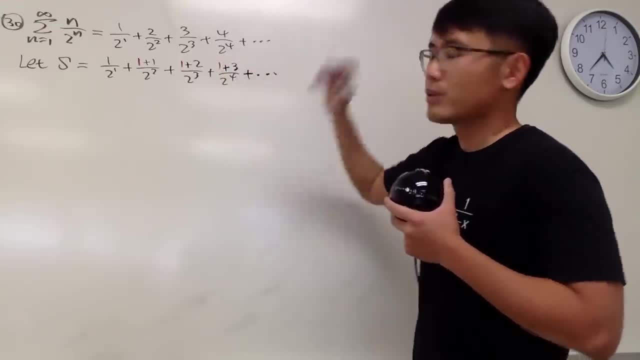 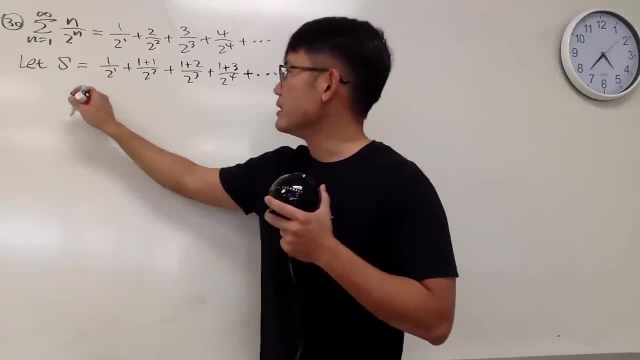 Of course, people will say: why don't you do 1 plus 1 plus 1 plus 1? No, Just don't. All right, Now we're going to play around with this. As you can see this right here, S will be the same as. 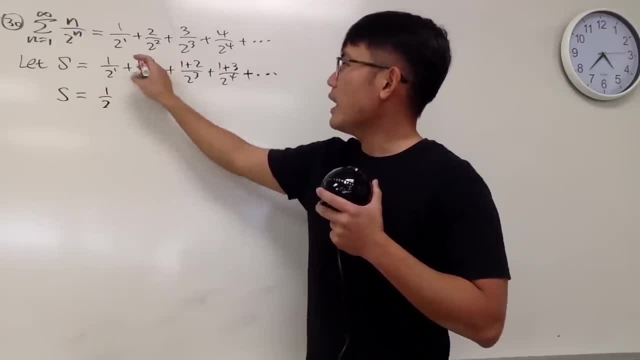 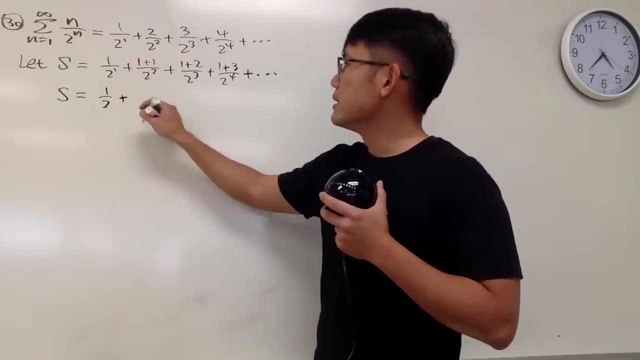 This is just 1 half, Just leave it. And now I will just leave this part in a second I will put this down right here- Plus 1 over. I'll just put everything in red. So 1 half plus. 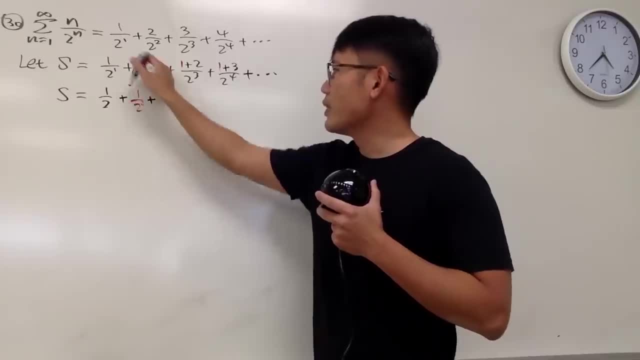 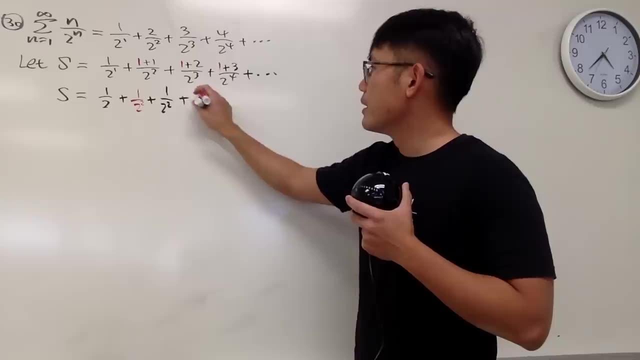 This is 1 over 1 over 2 squared, Sorry, 1 over 2 squared, And then 1 over 2 squared, again in black. And then this right here, plus 1 over 2 to the third power: 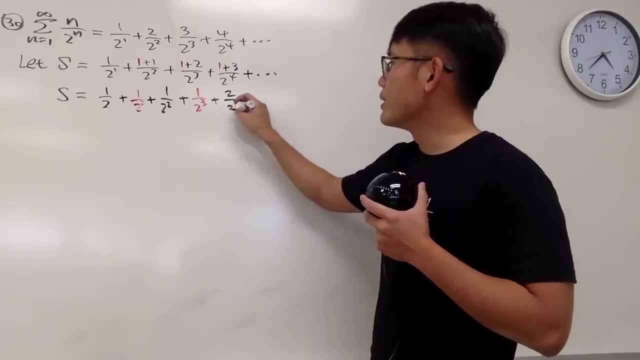 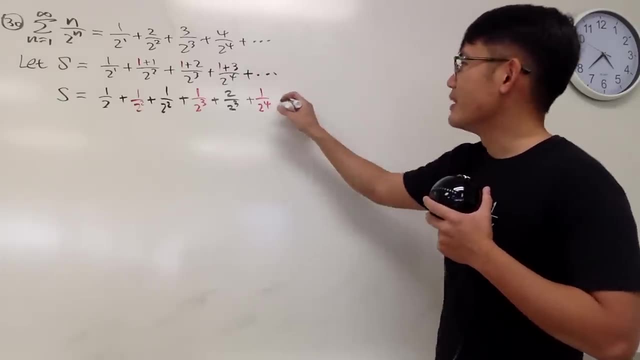 And then this right here is plus 2 over 2 to the third power. And then this right here is plus 1 over 2 to the fourth power. And then this right here is plus 3 over 2 to the fourth power. 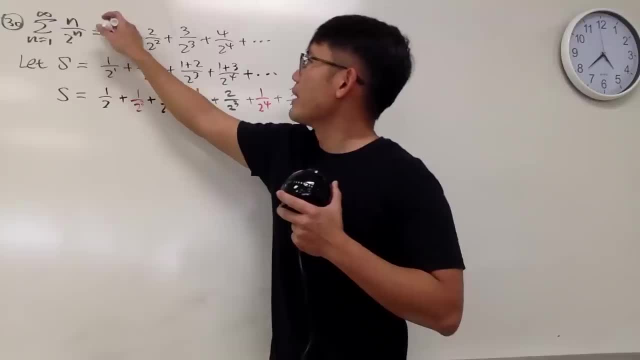 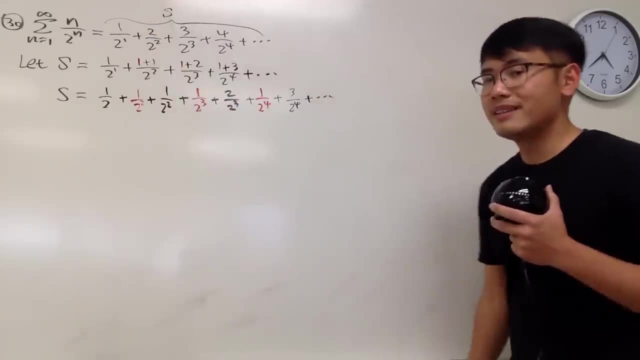 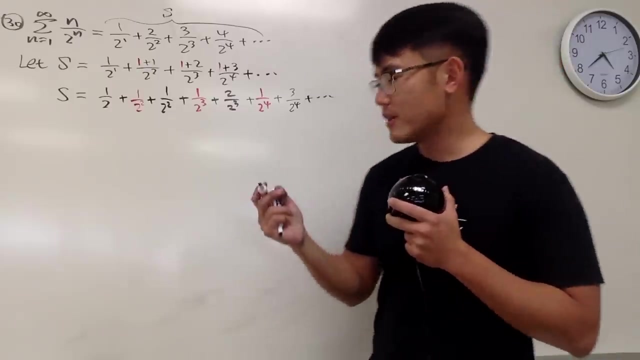 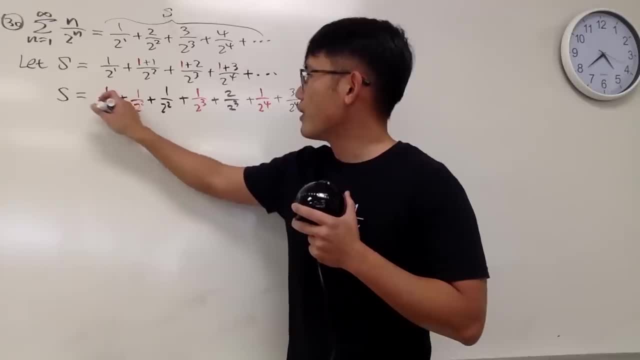 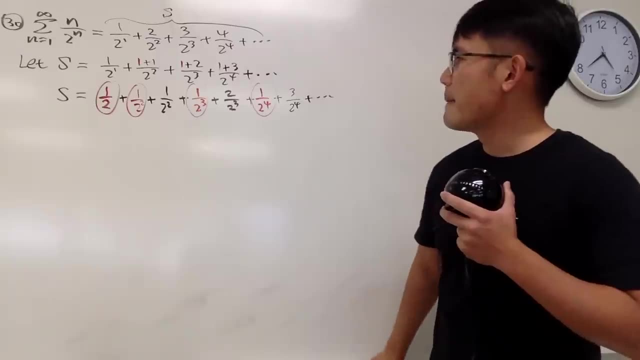 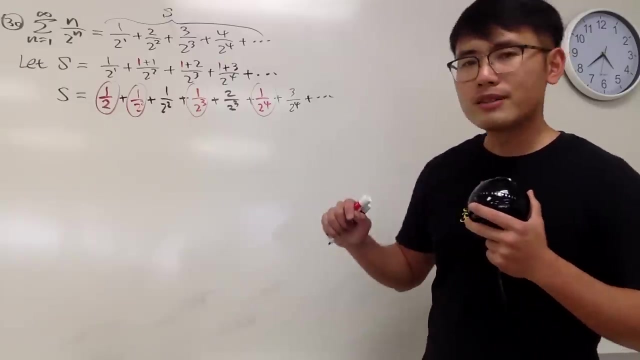 Okay, I know how to handle this. 1 over 2.. This is like this, this, this Looks good to me. The red parts are just the, you know the form of geometry series, And let's see, Let's do the math. 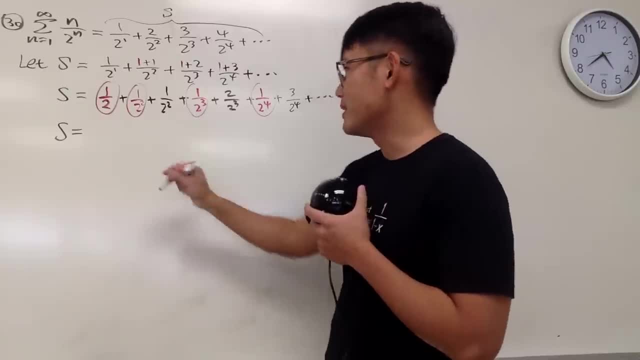 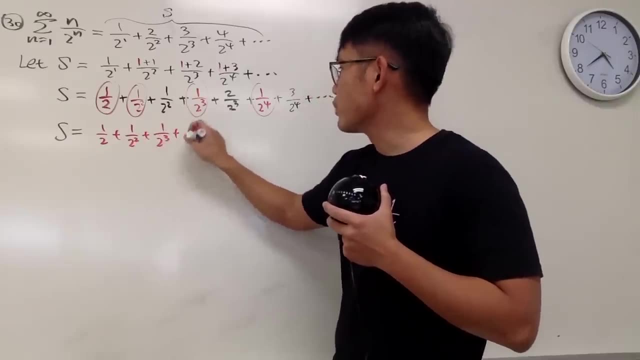 S is equal to. let me just put on red part first, so we can feel better. So I'll just put down 1 half, plus 1 over 2 to the second, plus 1 over 2 to the third, plus 1 over 2 to the fourth, plus, dot, dot, dot. 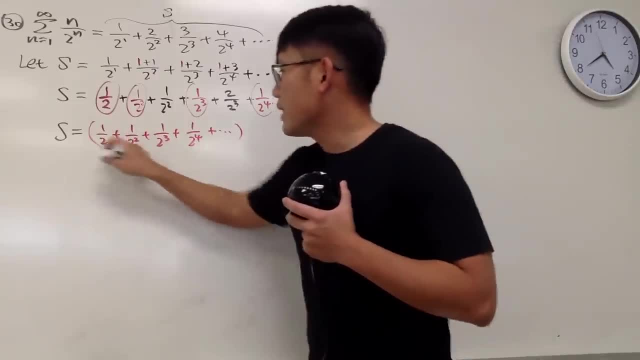 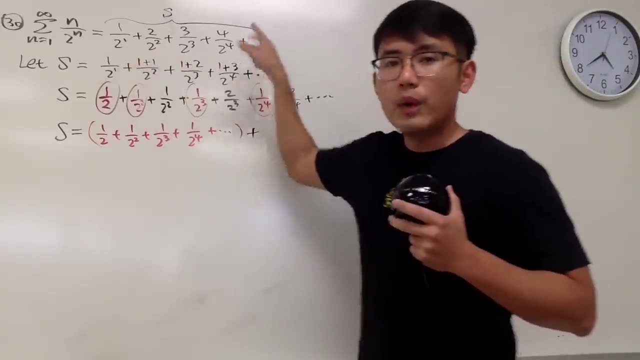 Because you know there will be other red parts as well. Okay, And then we add: Let's look at the parts in black. And if you look at the parts in black and compare this with the one that we did earlier, Hmm, Oh, look, look, look. 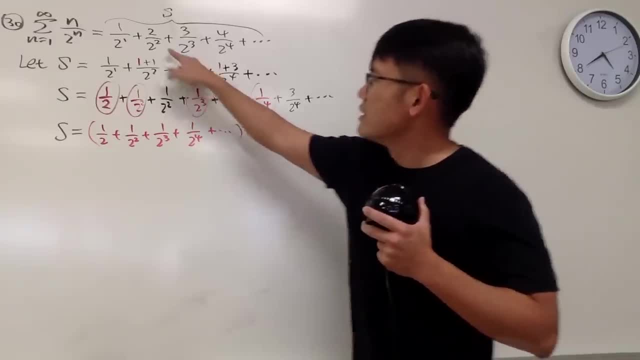 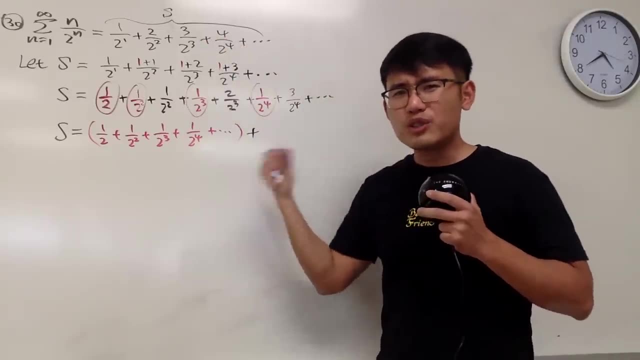 This is 2 over 2 to the third power, This is 2 over 2 to the second And this is 2 over 2 to the fourth, 3 and 3.. Maybe I should just factor out 2 in the denominator. 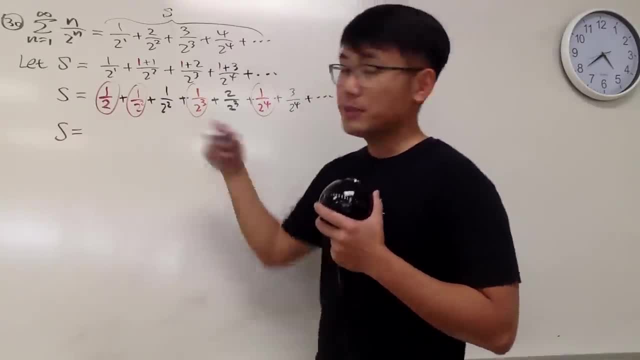 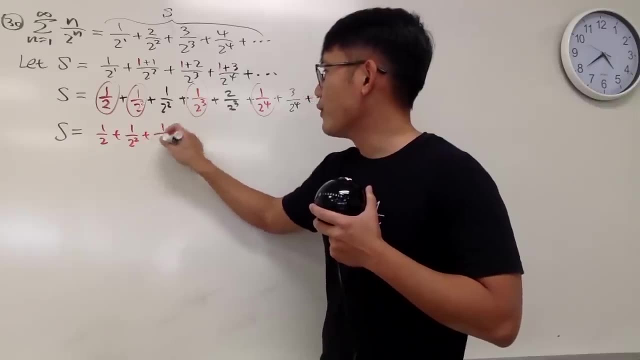 see, let's do the math. s is equal to. let me just put on grade proper so we can feel better. so I would just put down 1, 1 over 2 to the second, plus 1 over 2 to the third, plus 1 over 2 to the fourth, plus dot, dot, dot. 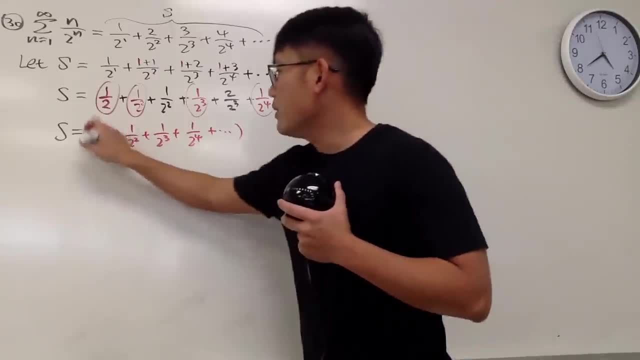 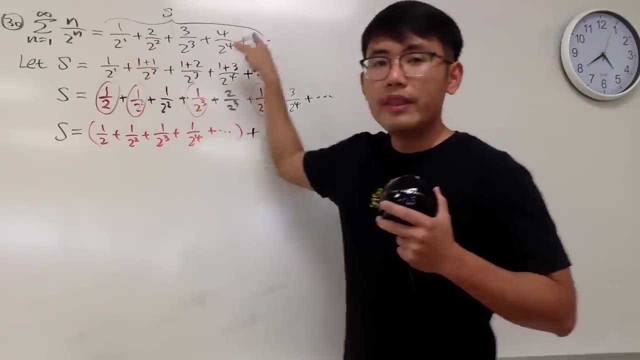 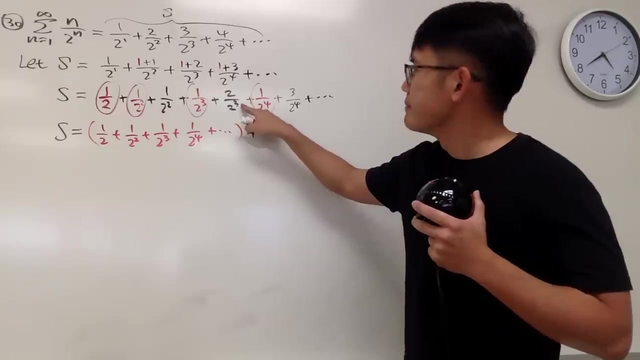 because you know there will be other red parts as well. okay, and then we add: let's look at the parts in black. and if you look at the parts in black and compare this with the one that we did earlier, hmm, oh, look, look, look. this is 2 over 2 to the third power. this is 2 over 2 to the second. 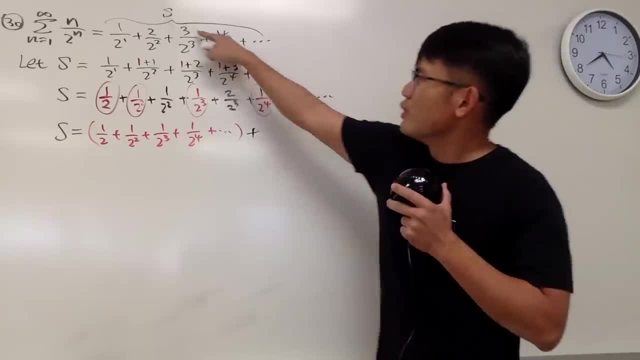 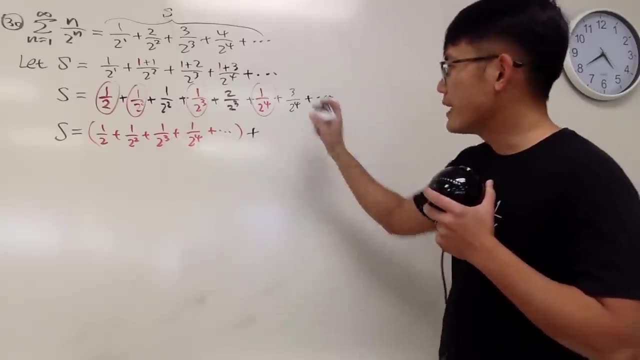 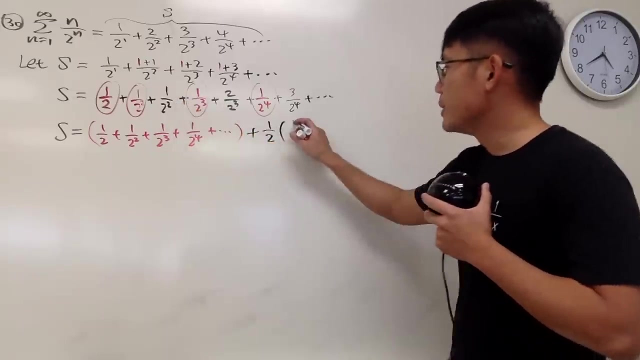 and this is 2 over 2 to the fourth, 3 and 3. maybe i should just factor out a 2 in the denominator. so pay attention to the bottom. i can factor out the one half. you know throughout the parts in black. so we see this is one half times. this guy is going to be 1 over 2 to the first, plus this. 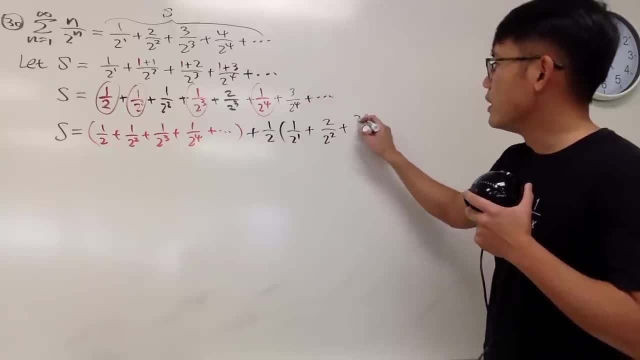 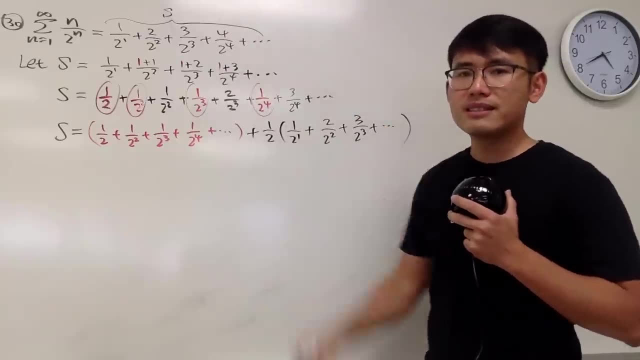 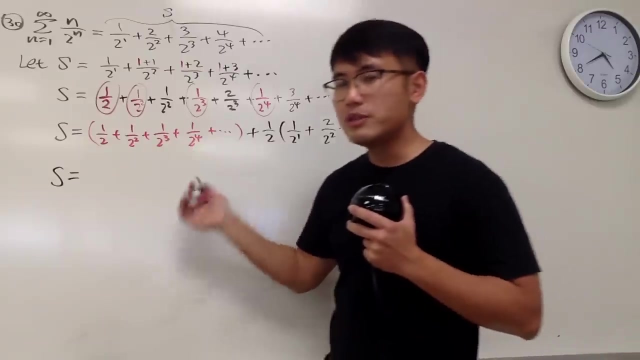 guy is going to be 2 over 2 to the second, and this guy is going to be 3 over 2 to the third, and then plus dot, dot, dot and so on, and guess what? this right here is just the same as n. very nice. well, now let's figure things out. s is still s, but this right here is a geometry series. 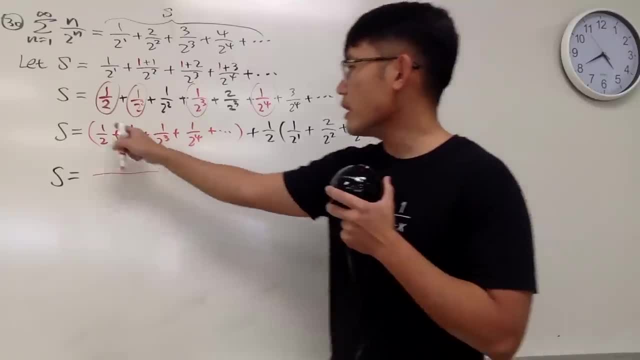 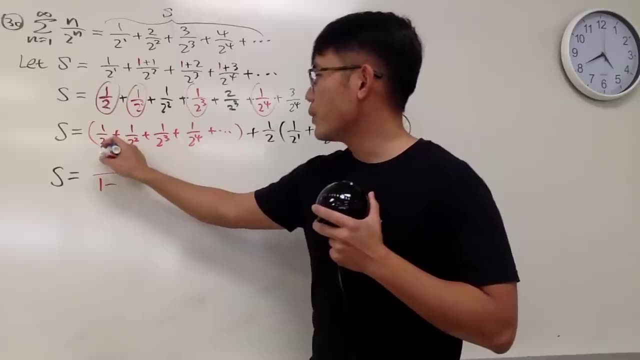 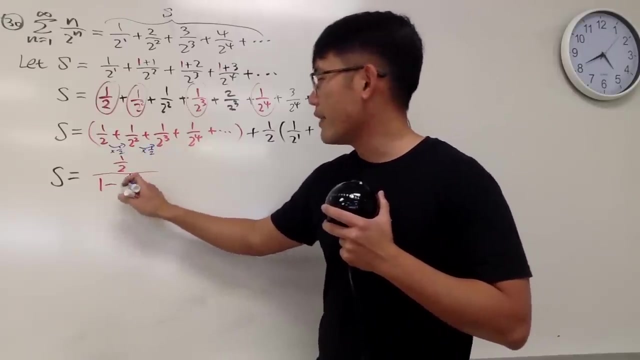 again, the best friend right here we can use the first one is just one half, the first time. just one half, and we have to do one minus, and when we go from here to here we multiply by one half. so that's the common ratio. so we will just do one minus one half, like that, and we will just have 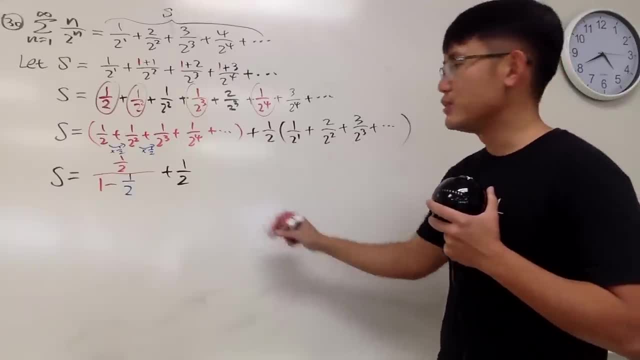 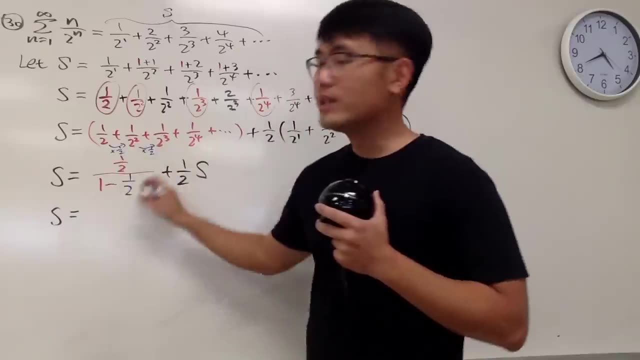 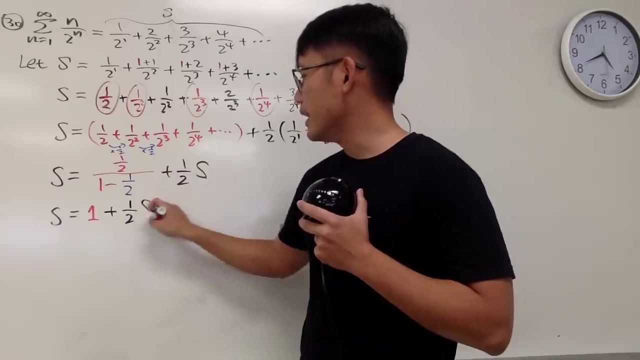 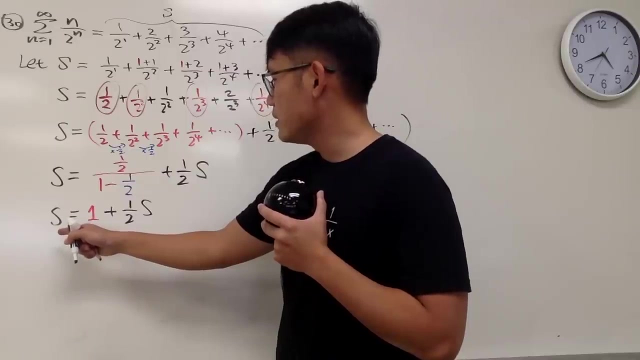 plus one half, but this guy is just the same as s. very cool, isn't it? now, s is equal to all this together is just a nice one, and this right here is plus one over two s, and of course, let's minus the s on both sides and we get this right here being one half s. 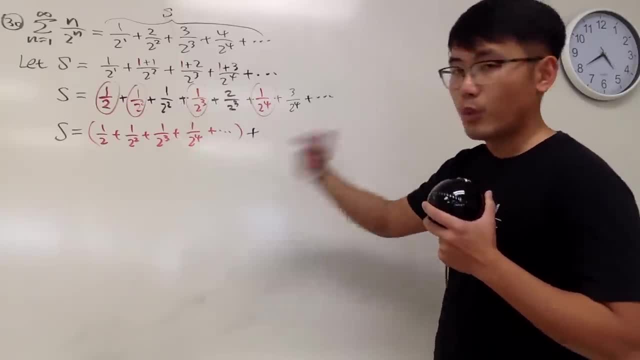 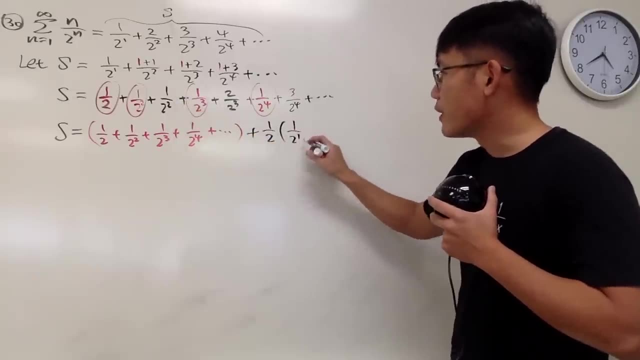 So pay attention to the bottom. I can factor out the 1 half. You know, throughout the parts Parts in black. So we see this is 1 half times. This guy is going to be 1 over 2 to the first, plus this guy is going to be 2 over 2 to the second. 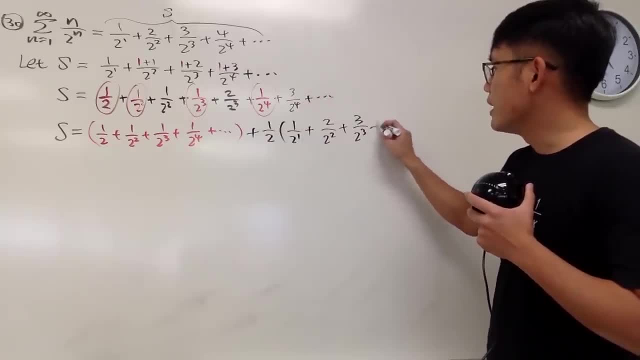 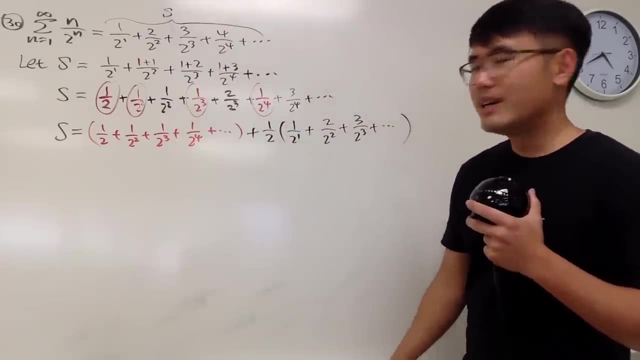 And this guy is going to be 3 over 2 to the third, and then plus dot, dot, dot and so on. And guess what? This right here is just the same as S. Very nice. Well, now let's figure things out. 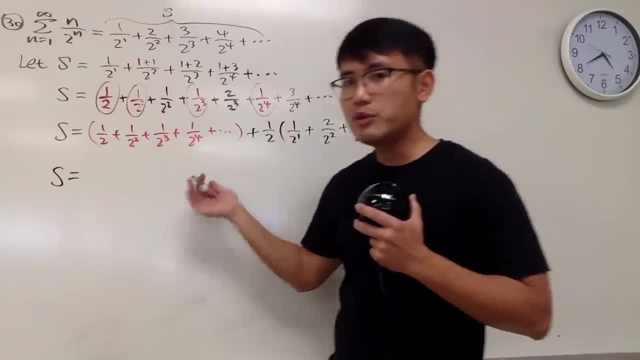 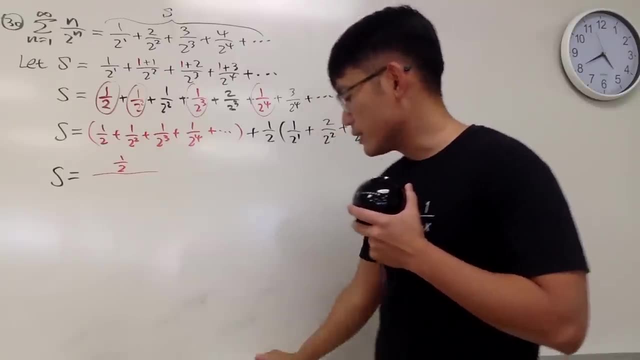 S is still S, But this right here is a geometric series. Again, the best friend right here we can use: The first one is just 1 half. The first one is just 1 half And we have to do 1 minus. 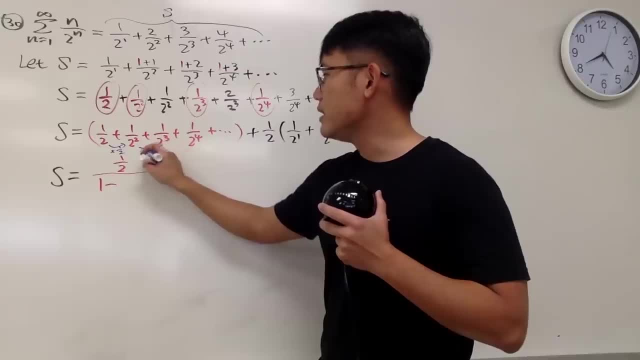 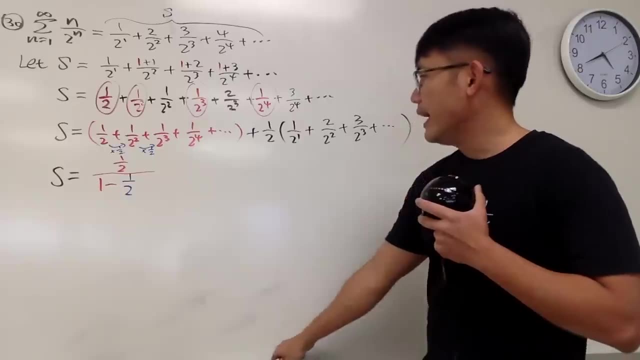 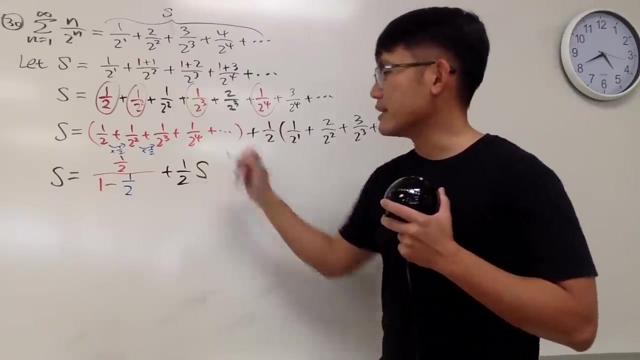 And when we go from here to here we multiply by 1 half. So that's the common ratio. So we will just do 1 minus 1 half like that, And we will just have plus 1 half. But this guy is just the same as S. 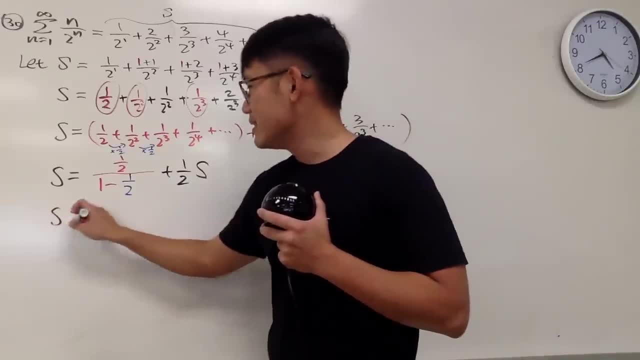 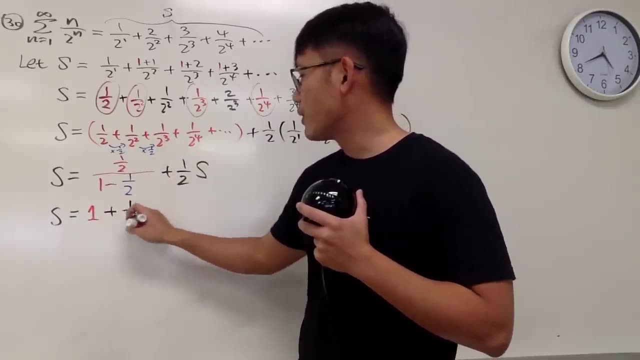 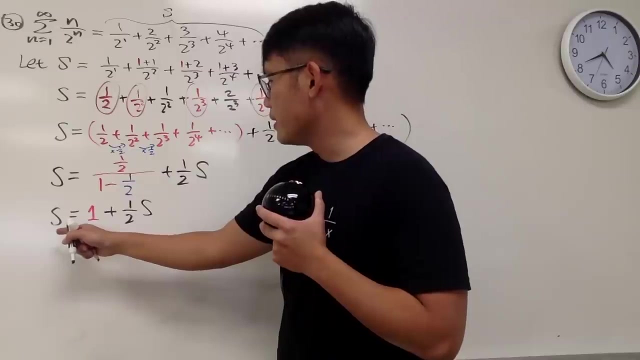 Very cool, isn't it? Now, S is equal to all this together is just a nice 1.. And this right here is plus 1 over 2S, And of course that's minus the S on both sides, And we get this right here being 1 half S. 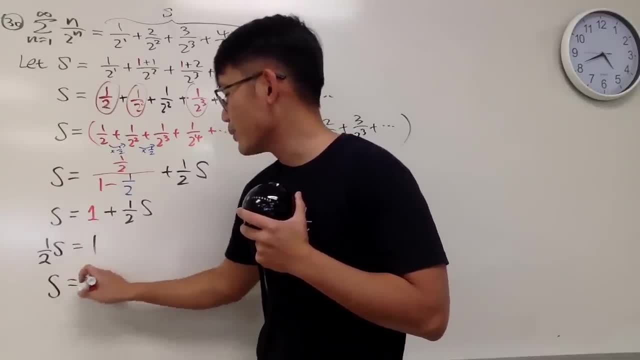 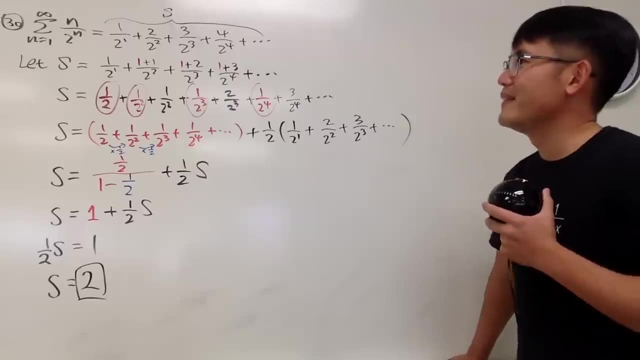 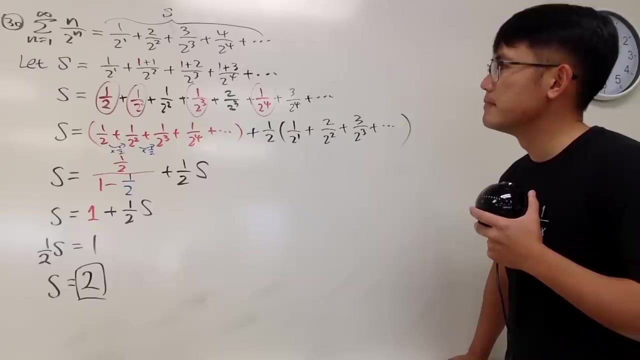 And that's equal to 1.. And, of course, in the end, S is equal to 2.. And with that we are done. Just like that. You're so good, Let's see. Yeah, I think that's it. 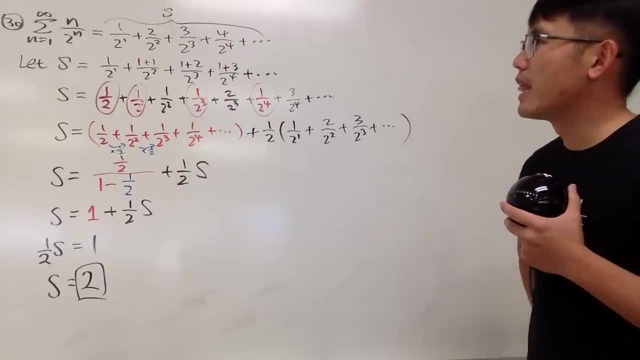 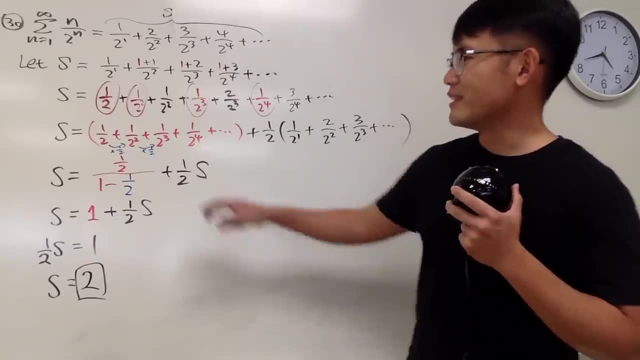 I think that's it. So, hmm, Oh yeah, of course I was thinking about, like how come this is bigger than the geometric sum? Of course, because the numerators are getting bigger and bigger. So that's it. 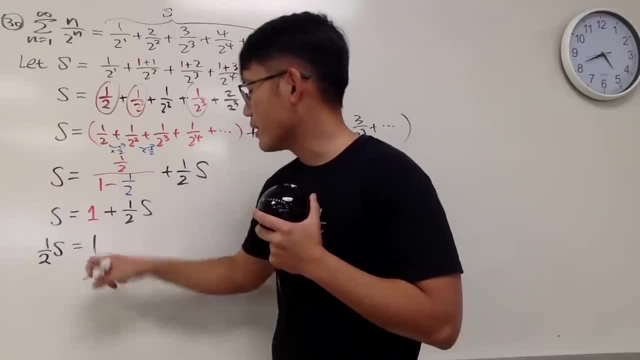 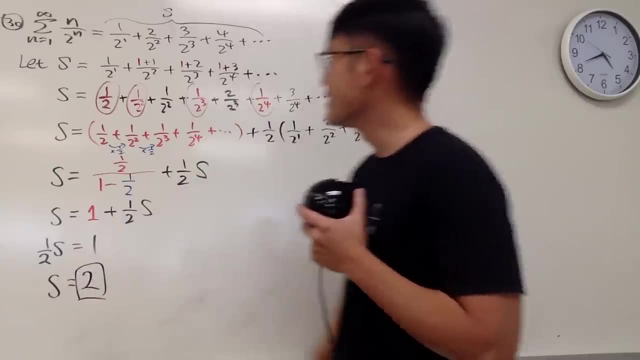 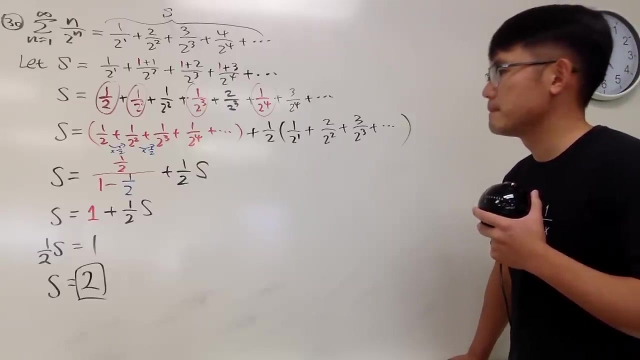 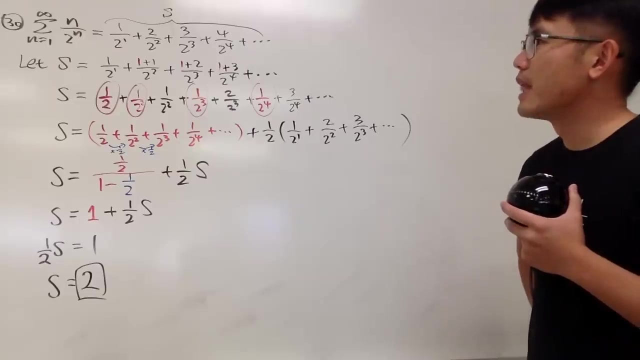 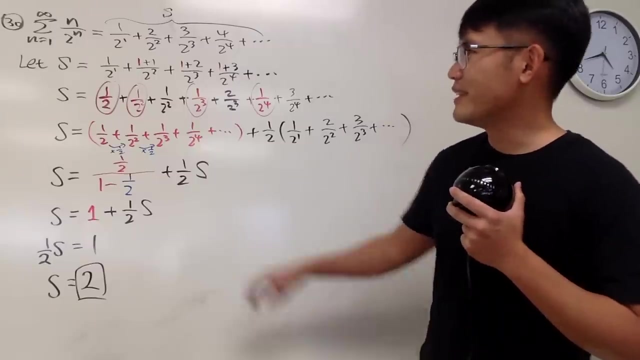 and that's equal to one and, of course, in the end, s is equal to two and with that we are done, just like that. huh, you're so good, let's see. yeah, i think that's it right, i think that's it so. hmm, oh yeah, of course i was thinking about, like how come this is bigger than the geometric? 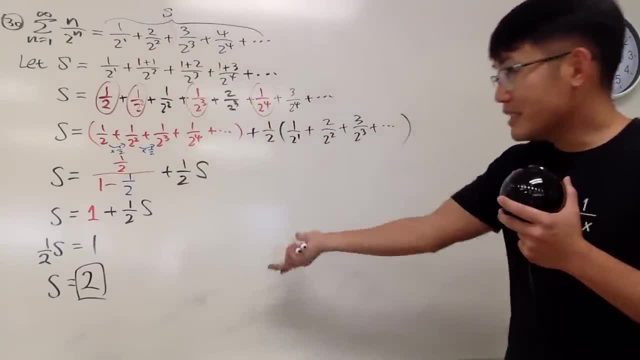 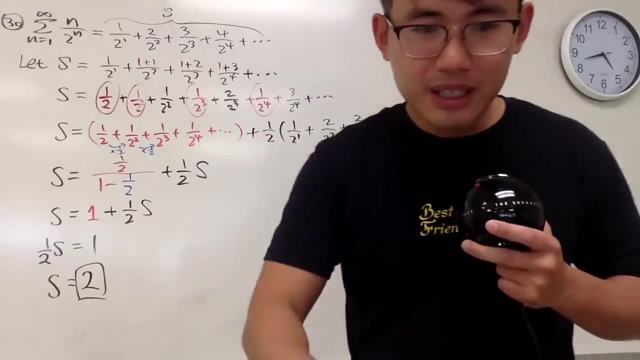 sum, of course, because the numerators are getting bigger and bigger. so that's it. that's it seriously. that's it all right, that's it's true. i know you see a lot of tools, but like the answer is also two, so not my fault, just two. 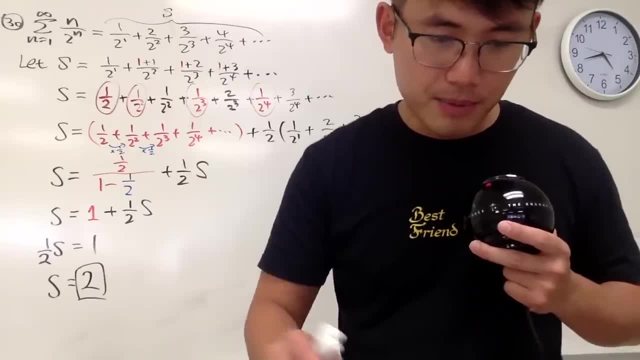 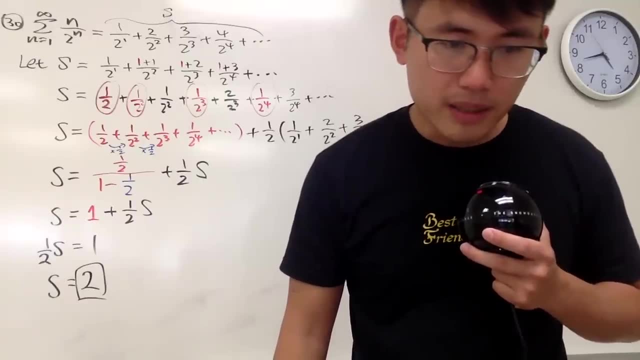 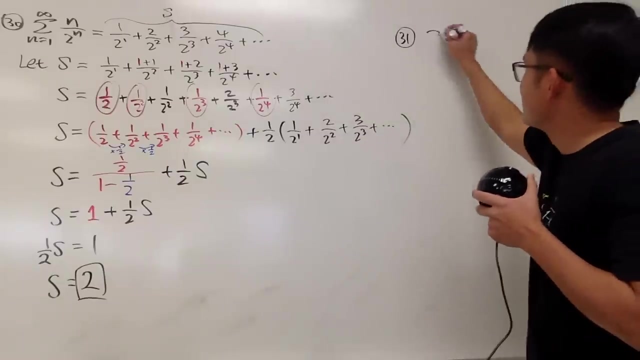 Okay, Number 30,. no, let's do number 31.. So let's look at number 31, right here For number 31,. we have this big giant fraction. Let's see, We have to do the sum as n goes from 1 to infinity. 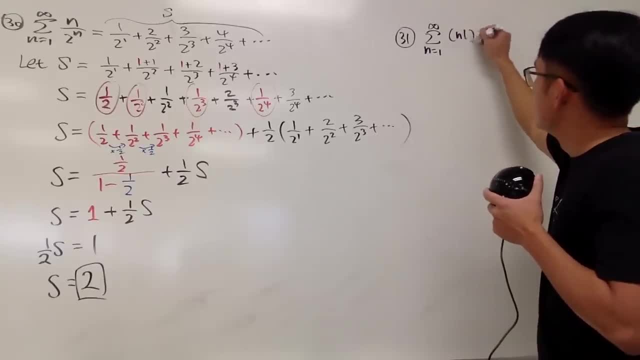 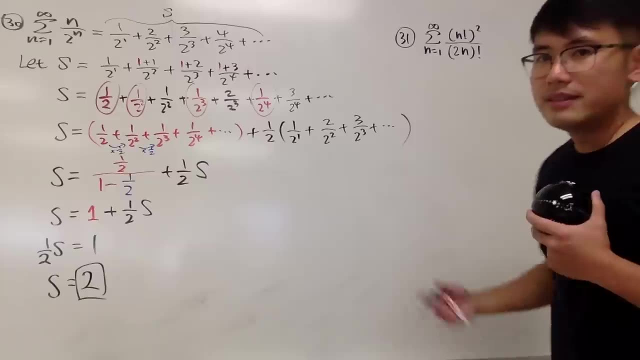 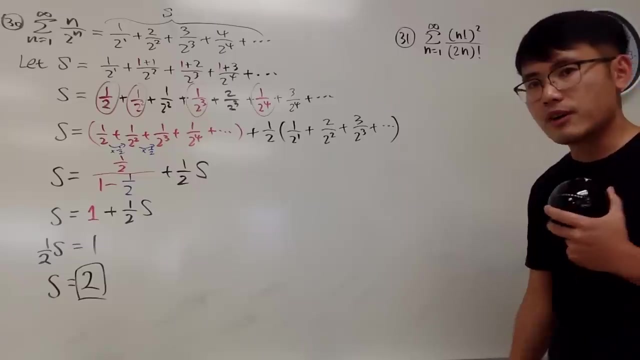 and then we have n factorial square over 2n, and then factorial right. This is actually a pretty famous one, so let's go ahead and do this, All right? So we see factorial. so the good idea is just use the ratio test. 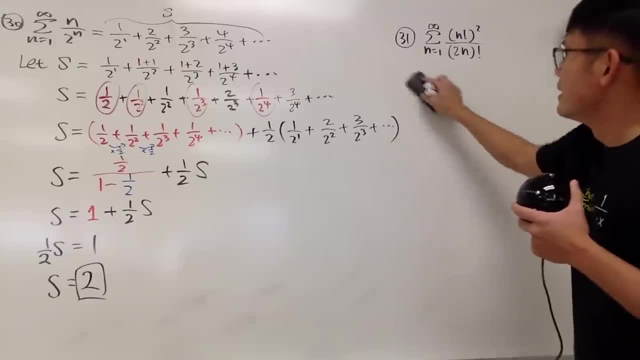 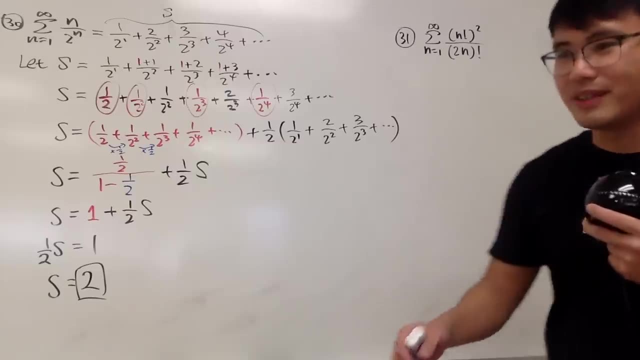 So here we go. We are going to check the limit as x as n goes to infinity, right, So I'm not going to pick it out. I have a lot of these, so don't worry. All right, So here we go. I will just say: 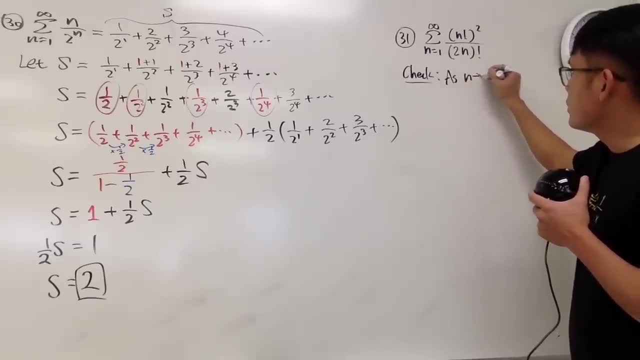 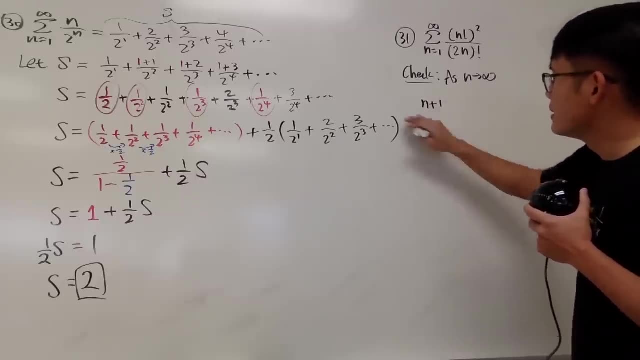 we are going to check and I will just do as n goes to infinity. Well, I'm going to put in n plus 1 to all the n's. So here we get n plus 1, and let me just erase n plus 1,. 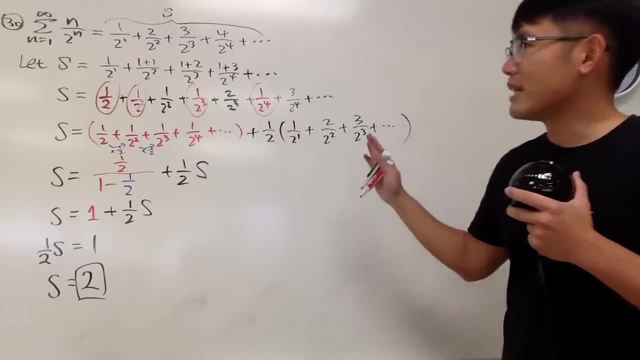 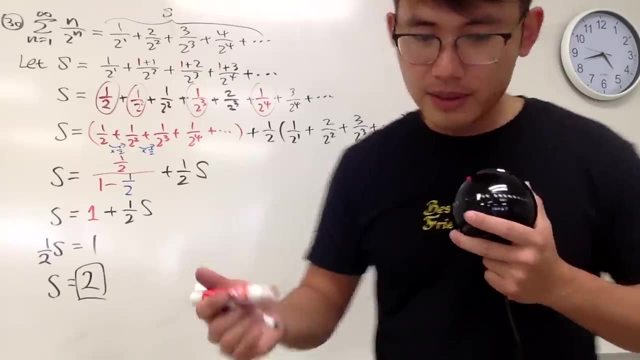 That's it Seriously. that's it. The answer is 2.. I know you see a lot of 2s, but like the answer is also 2. So not my fault, Just 2.. OK, Number 30.. 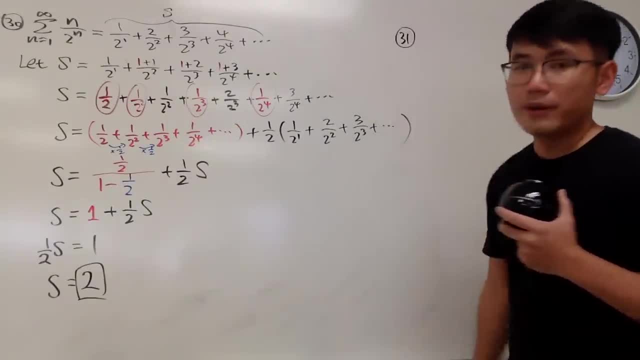 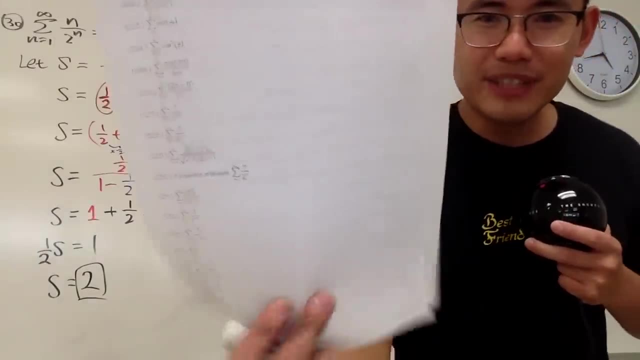 No, let's do number 31.. So let's look at number 31, right here For number 31, we have this big giant fraction. Let's see, We have to do the sum, as n goes from 1 to infinity. 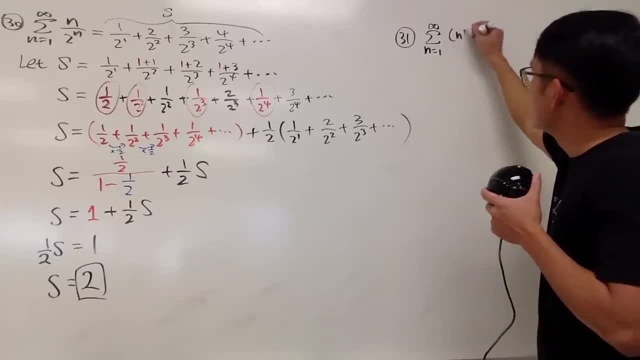 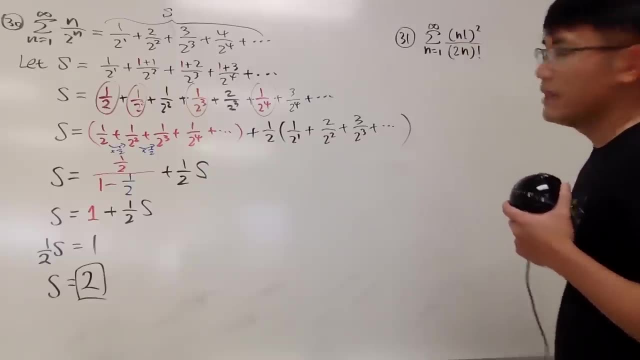 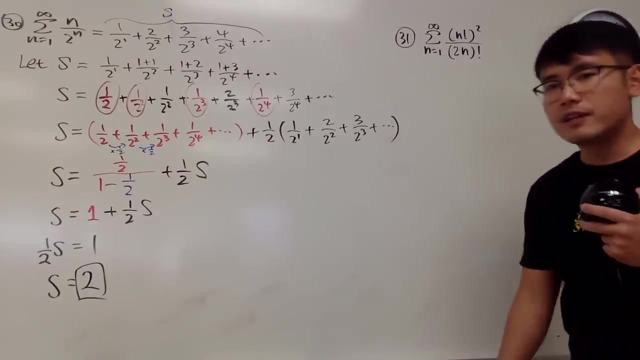 And then we have n factorial squared over 2n, and then factorial Right. This is actually a pretty famous one, so let's go ahead and do this. All right? So we see factorial. so the good idea is just use the ratio test. 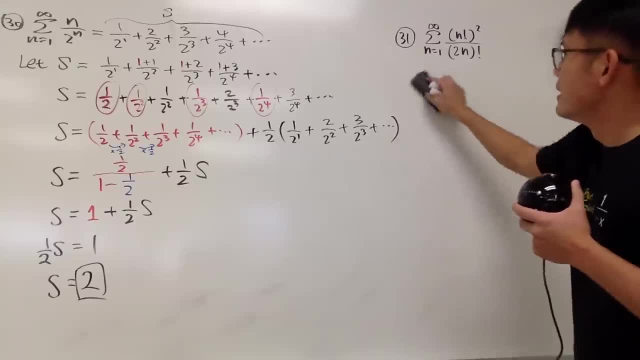 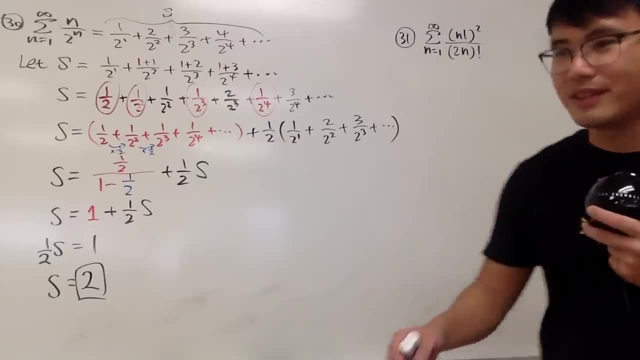 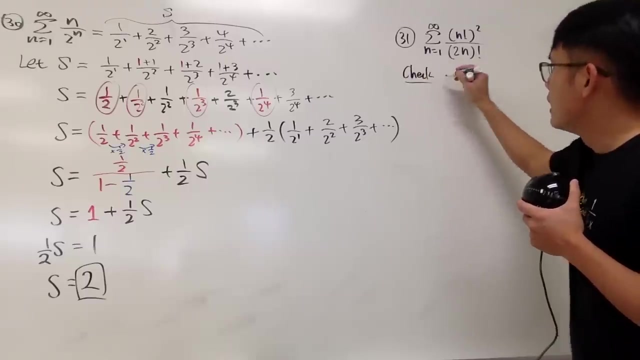 So here we go. We are going to check the limit as n goes to infinity, Right? So I'm not going to pick it out. I have a lot of these, so don't worry, All right. So here we go. I will just say we are going to check and I will just do as n goes to infinity. 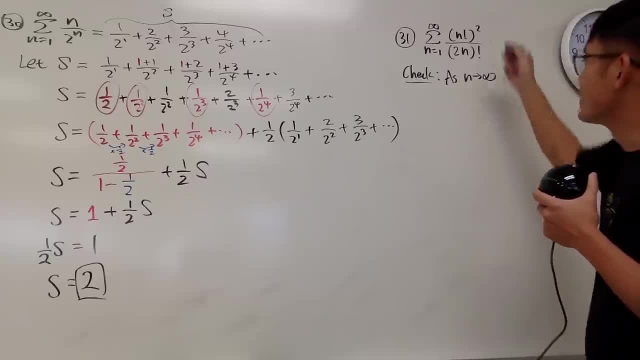 Well, I'm going to put in n plus 1 to all the n's. So here we get n plus 1, and let me just erase n plus 1,, and then you do the factorial, and then we do the square. 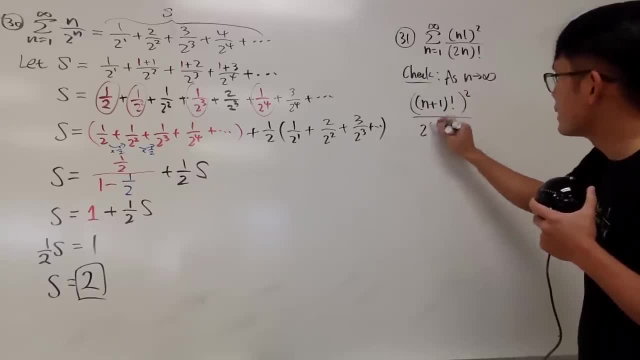 And then we put the n plus 1 right here as well, So we have over 2 times n plus 1 in the parentheses like this. And then the factorial is actually on the outside And technically we still have to do the absolute value. 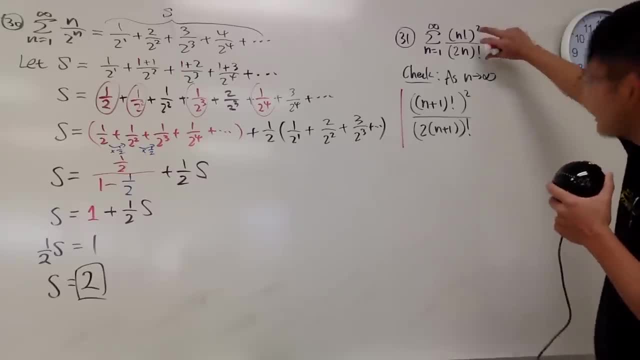 Right, So this is the a, n plus 1.. Now let's take this and multiply by the reciprocal, So we get 2n factorial over n factorial and we square that like this. And now it's just hard to work this out. 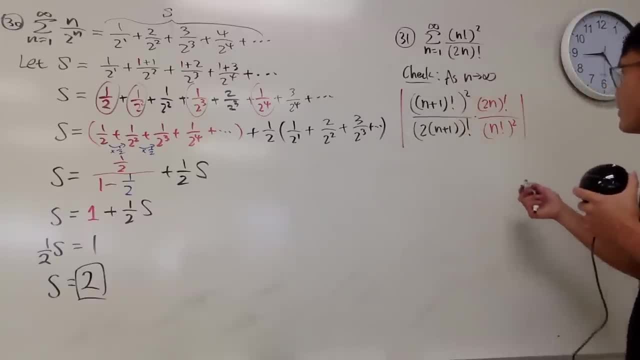 Usually people like the ratio test a lot because it's a lot of computations. So let's see: OK, Inside, here we can write this as n plus 1 square because of the square, And next we have the n- factorial and square. 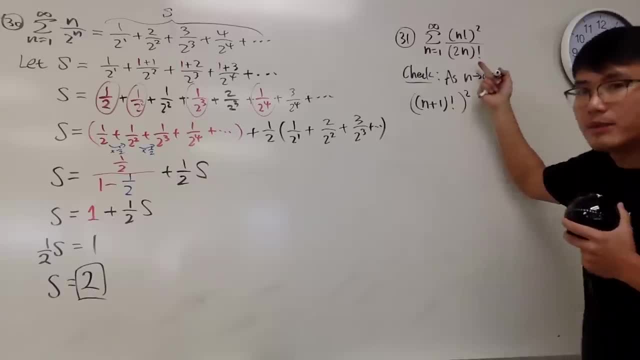 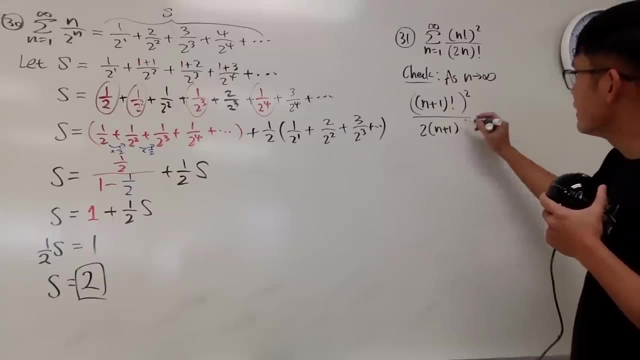 and then you do the factorial, and then we do the square, and then we put the n plus 1 right here as well. So we have over 2 times n plus 1 in the parentheses like this, and then the factorial- it's actually on the outside. 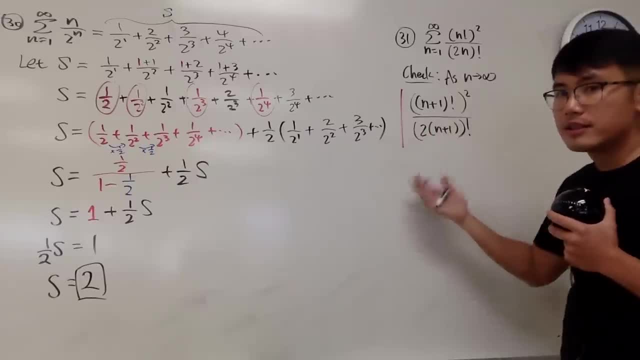 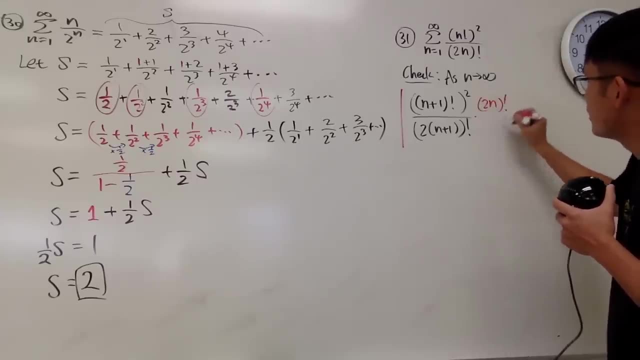 And technically we still have to do the absolute value right. So this is the a, n plus 1.. Now let's take this and multiply by the reciprocal, so we get 2n factorial over n factorial and we square that like this: 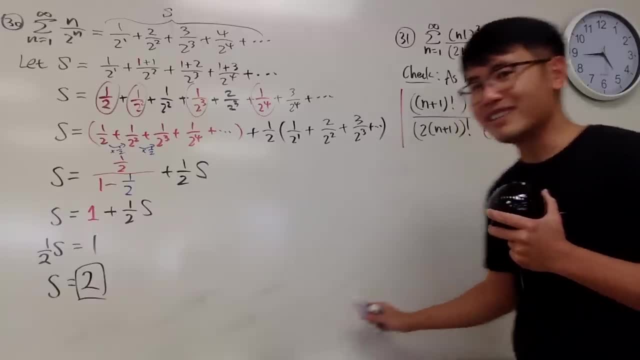 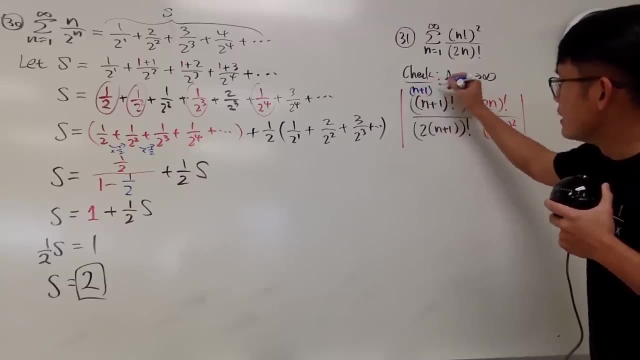 And now it's just hard to work this out. Usually people like the ratio test a lot because it's a lot of computations. So let's see, Okay, Inside here we can write this as n plus 1 square because of the square. 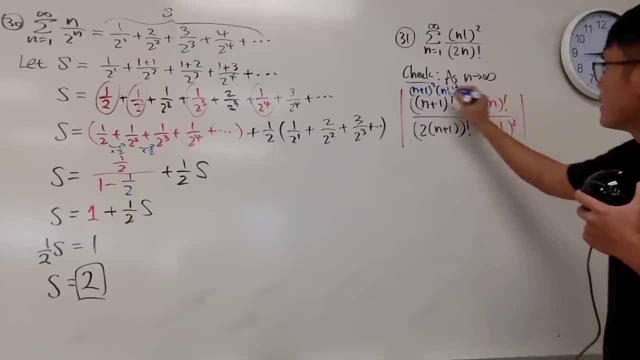 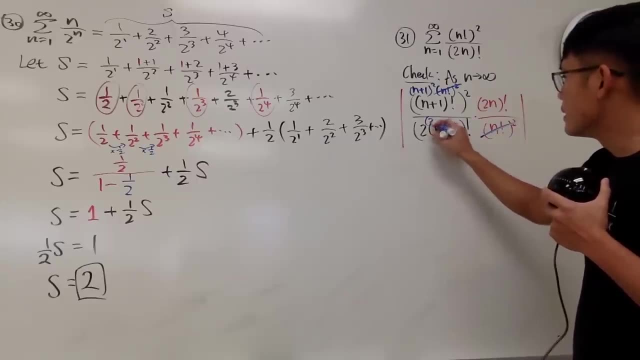 and next we have the n- factorial and square, and again this, and that can also be cancelled out. Now for this guy, this is, of course, 2n plus 2 factorial. So to break this down, this is how we do it. 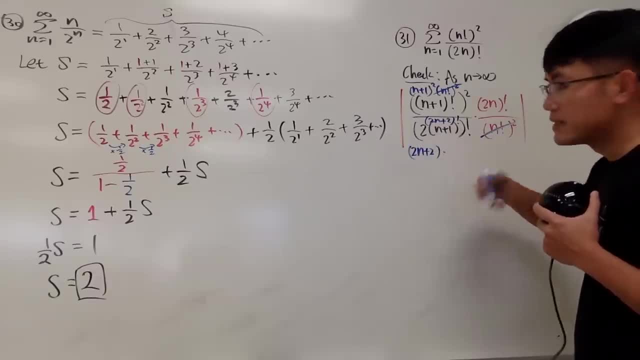 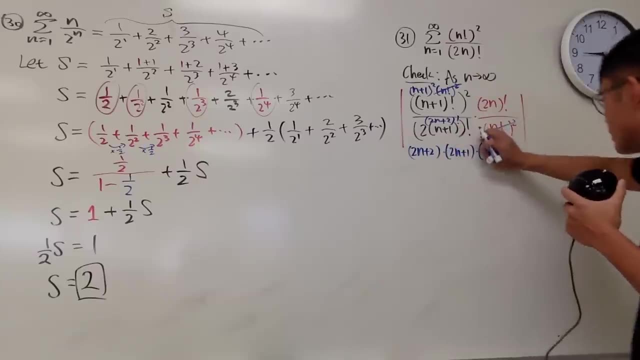 We start with 2n plus 2 times the next number, which is 2n plus 1, times the next number, which is 2n, and we're going to stop because you know it can keep on going forever. 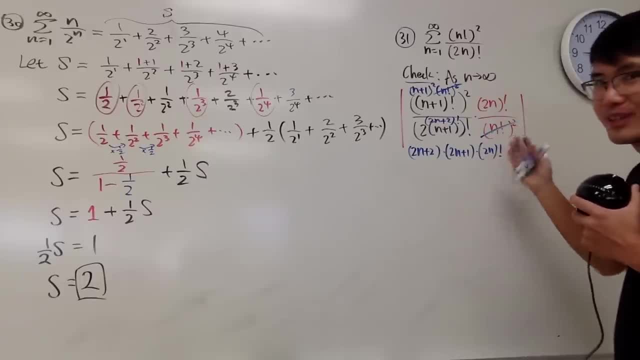 Well, not forever, until 1.. And then you have the factorial right here. That's why you can stop right here. The good thing is this and that can be cancelled. So that's nice, and I think that's what we have right. 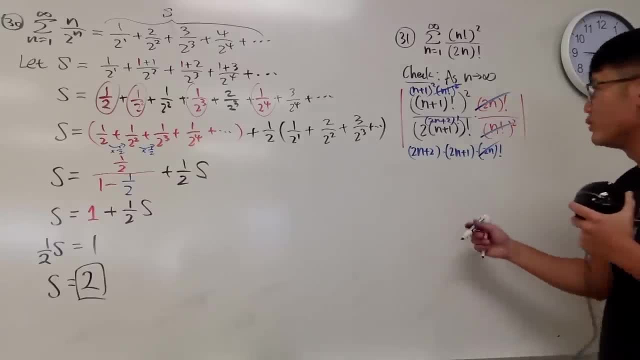 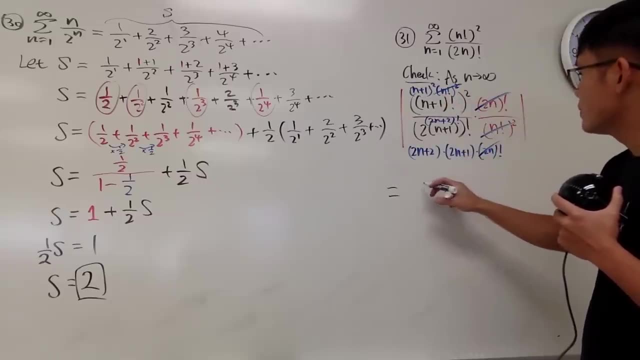 So we are just going to do the rest of the algebra. On the top we have n plus 1 square, So we can just multiply. Let me just write it down again to make it clear: n plus 1 square over this is 2.. 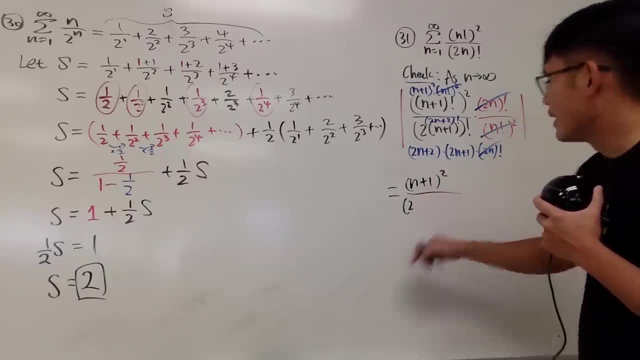 Okay, I can factor out the Why not. This is just algebra. I can factor out the little 2 right here: okay, So 2n plus 1, and then this right here is 2n plus 1.. So you can cancel this guy and that guy out. 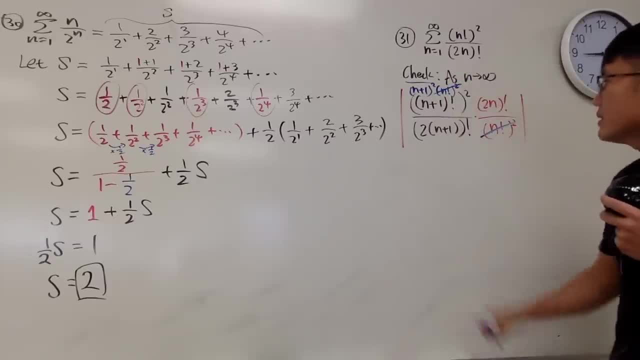 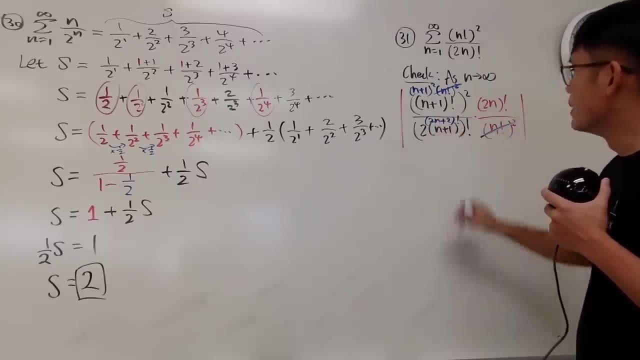 And again this and that can also be canceled out. Now, for this guy this is of course 2n, So 2n plus 2 factorial. So to break this down, this is how we do it: We start with 2n plus 2 times the next number, which is 2n, plus 1 times the next number, which is 2n. 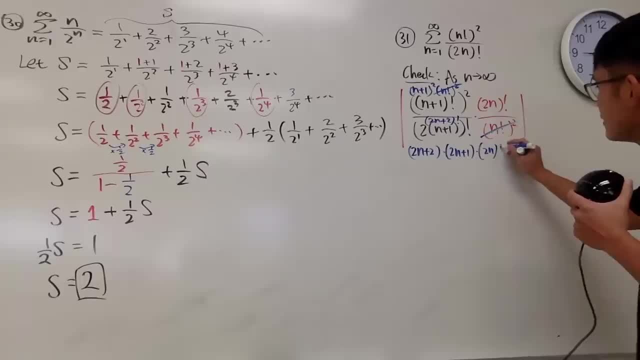 And we are going to stop because you know it can keep on going forever. Well, not forever, until 1.. And then you have the factorial right here. That's why you can stop right here. The good thing is this: and that can be canceled. 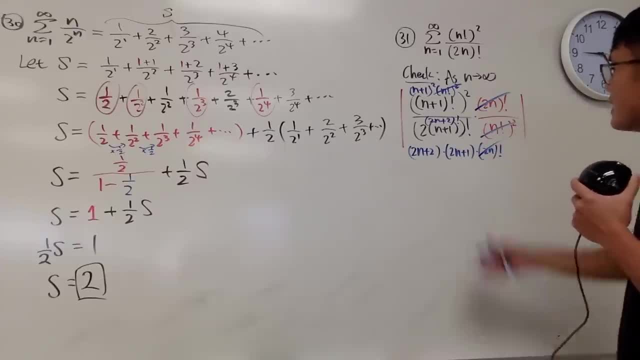 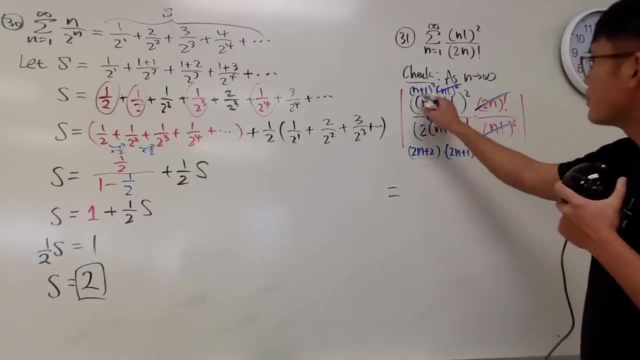 So that's nice And I think that's what we have. All right. So we are just going to do the rest of the algebra. On the top we have n plus 1 square, So we can just multiply. Let me just write it down again to make it clear. 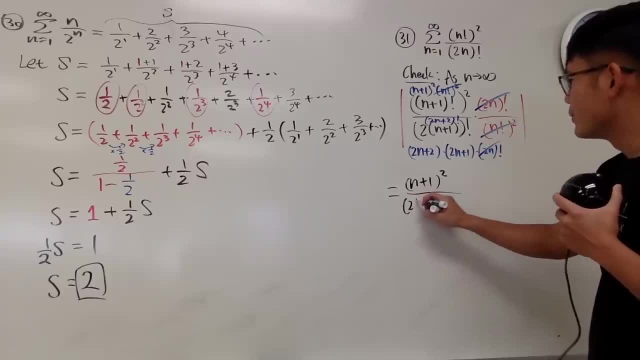 n plus 1 square over, this is 2.. OK, I can factor out the point. now. This is just algebra. I can factor out the little 2 right here. OK, So 2n plus 1.. And then this right here is 2n plus 1.. 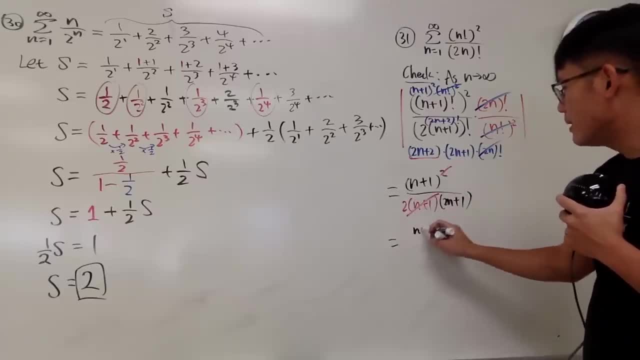 So you can cancel this guy and that guy out. So you get n plus 1 over Distribute, We get 4n plus 2, like this: Yeah, What's the limit? Approaches 1 over 4.. Why? 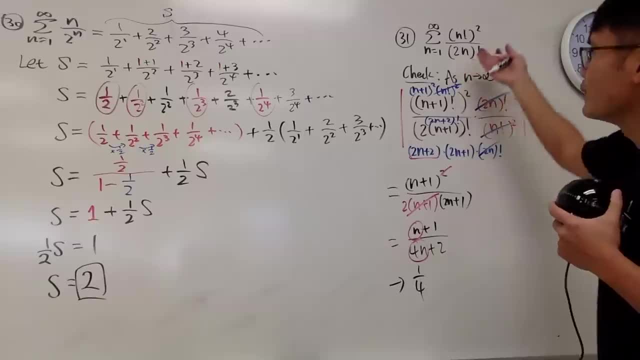 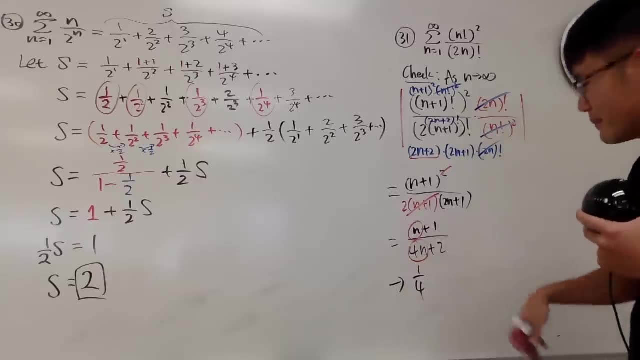 This and that. Right, The dominating part, OK. Finally, you see that a ratio test actually ends up with a limit Not equal to like 1 over 2.. Well, actually I'm talking about no, never mind. 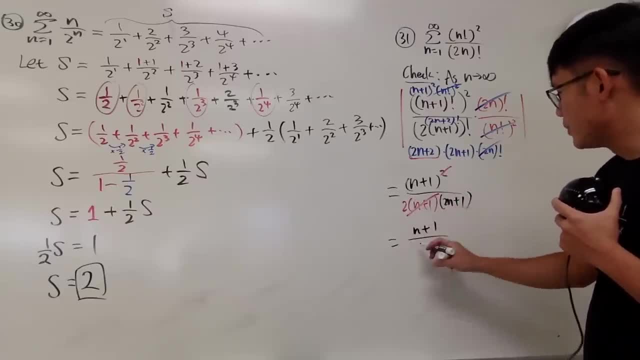 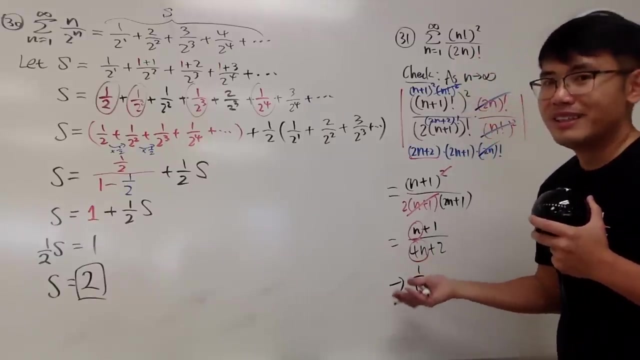 So you get n plus 1 over distribute we get 4n plus 2, like this: Yeah, What's the limit? Approaches 1 over 4.. Why This and that right, The dominating part? Okay, finally, you see that a ratio test actually ends up with a limit not equal to like 1 over 2.. 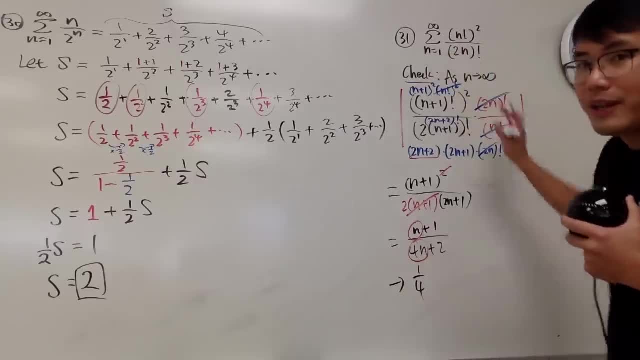 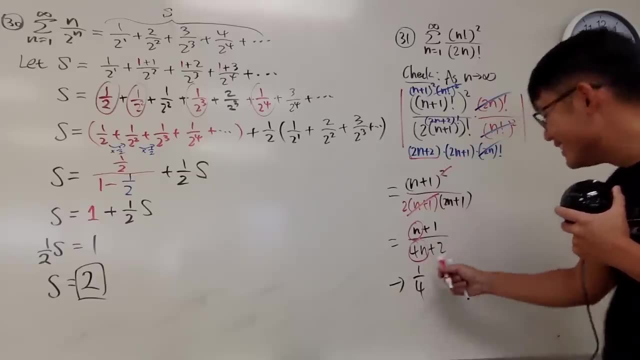 Well, actually I'm talking about No, never mind This right here. it's not like ending on 0 or whatever. so, But you have to pay attention to the limit that we get from the ratio test. This has to be less than 1 or bigger than 1 to draw a conclusion. 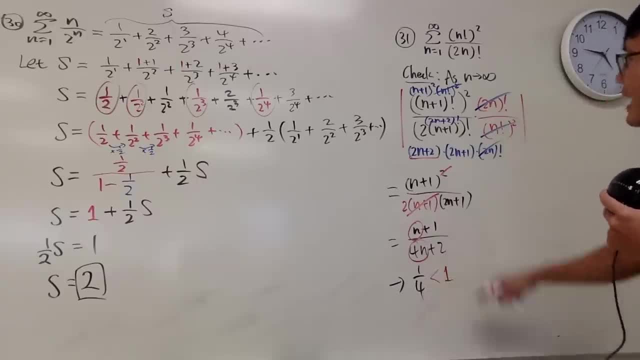 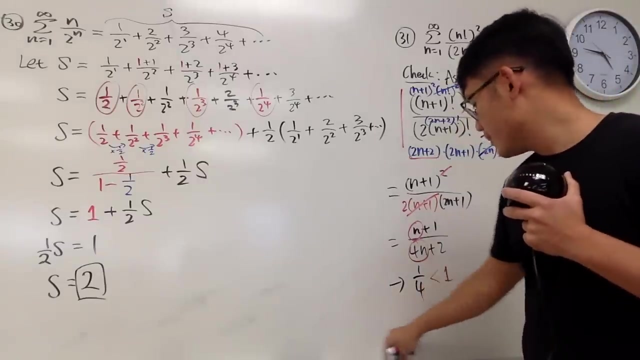 1 will be useless for the ratio test, But less than 1 tells us that this right here Converges, And again, let's say, by the ratio test, Right? So just like that. Whew, It's a lot of fun for that one. 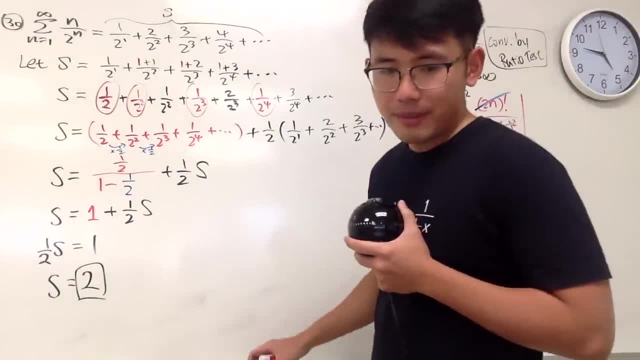 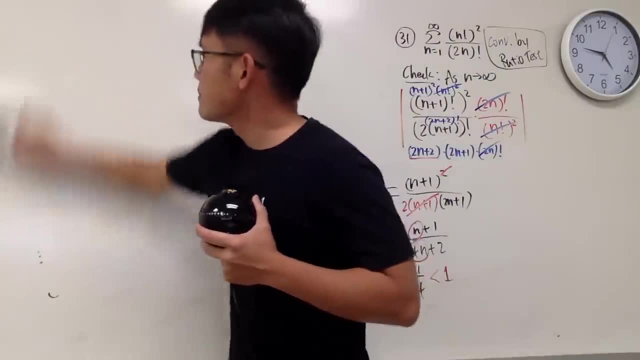 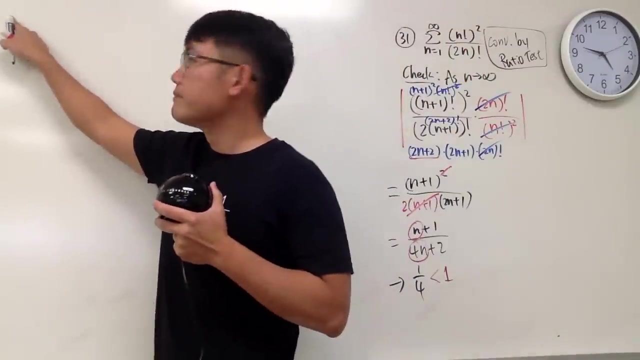 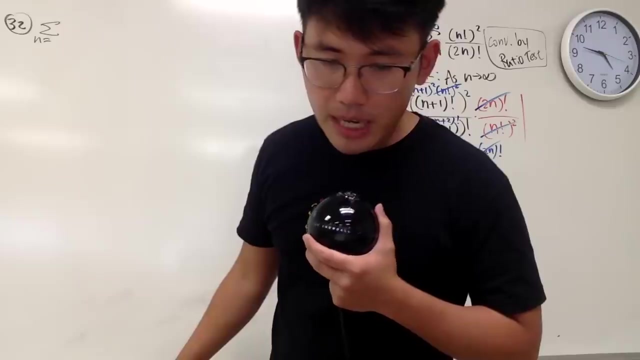 Okay, Now Okay, Number 32 and number 33,. again, I'm going to do them side by side. I will do them side by side and we'll see how it goes. So we have 1 to infinity And then we have 1 over. 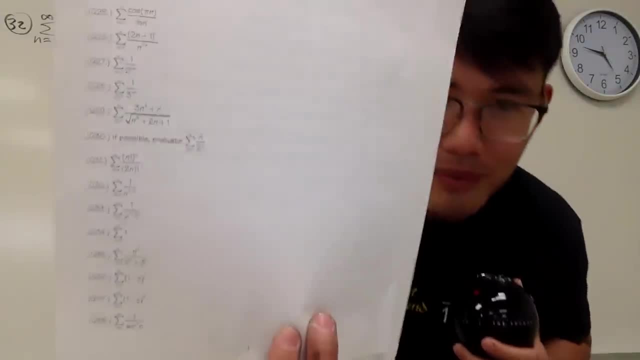 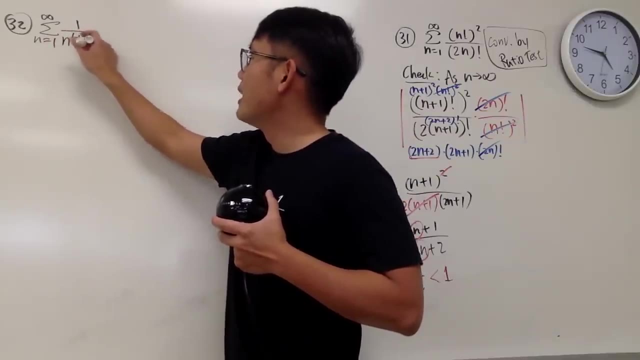 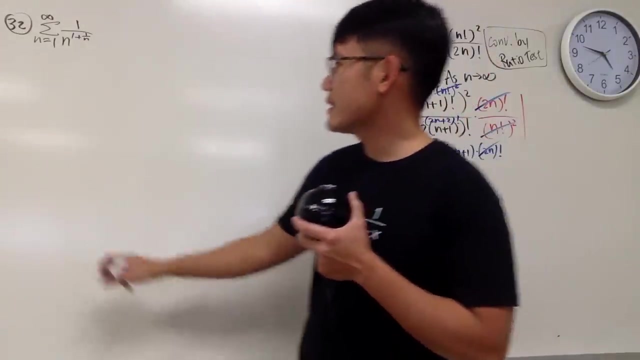 And we have n to the 1 over 1.. n to the 1 plus Oh man, n to the 1 plus 1 over nth power, like that. Hmm, Right, And actually let's just focus on this one first. 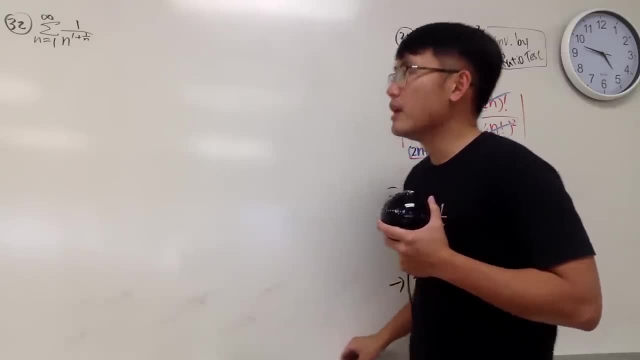 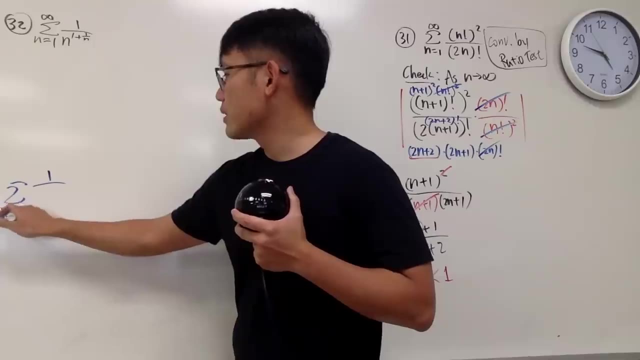 First of all, this is a common mistake for this question. A lot of people will just think that, okay, here we have 1 over the sum, as n goes from 1 to infinity. And okay, we have 1 over n plus 1 over n. 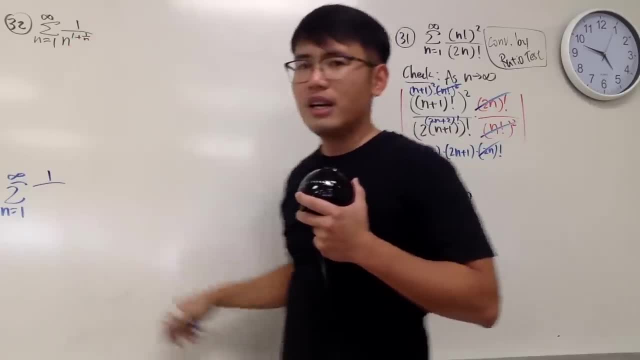 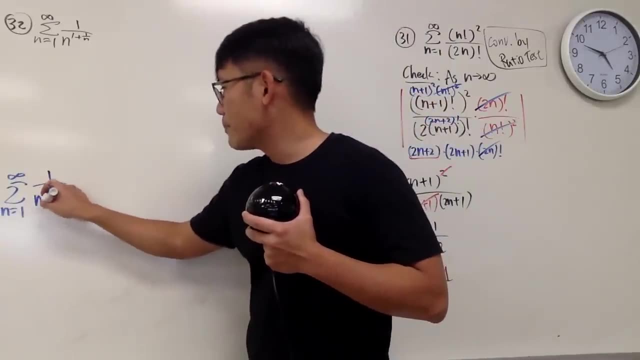 So the numerator, It's not a numerator. The power: right here it's bigger than 1.. This is a common mistake. You can just- You cannot just- do n to the 1 plus 1 over n and say this: right here is the p which is greater. 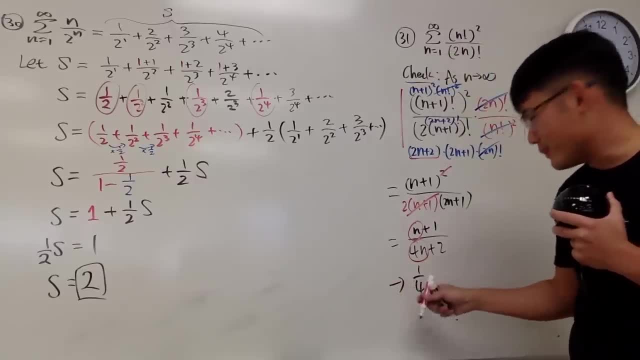 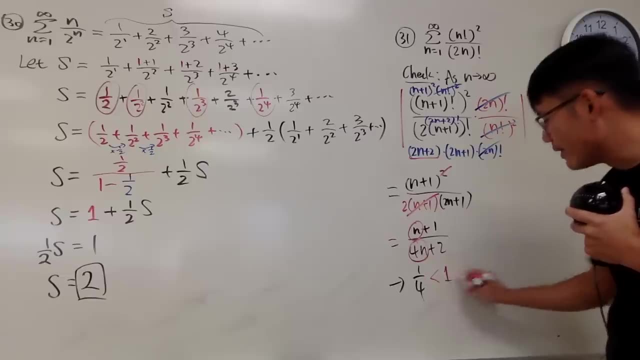 This right here. it's not like ending on 0 or whatever. So, but you have to pay attention to the limit that we get from the ratio test. This has to be less than 1 or bigger than 1. to draw a conclusion, 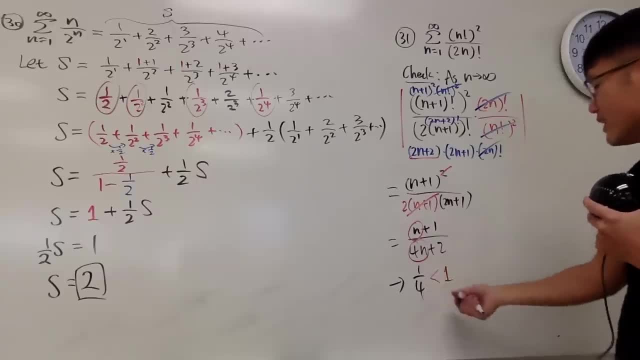 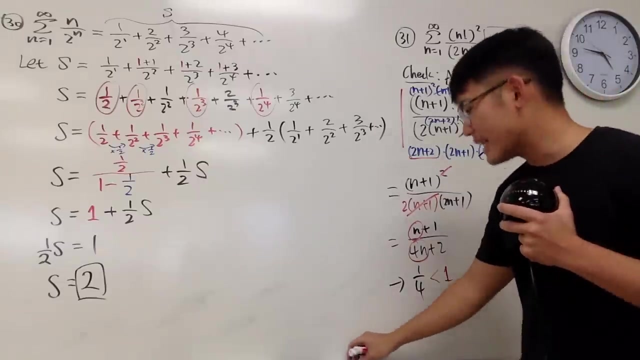 1 will be useless for the ratio test. But less than 1 tells us that this right here converges, And again, let's say, by the ratio Ratio test, Right, So just like that. Whew, It's a lot of fun for that one. 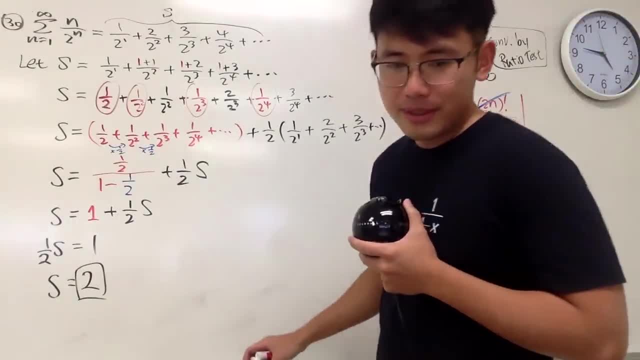 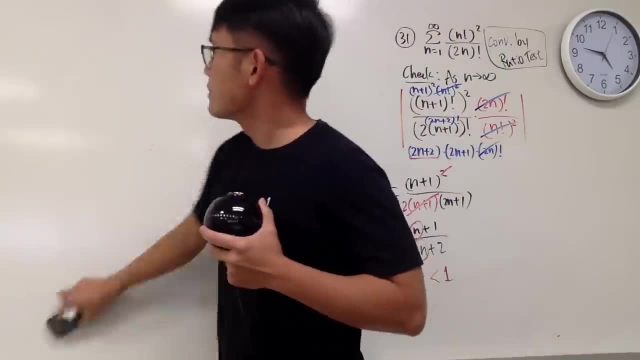 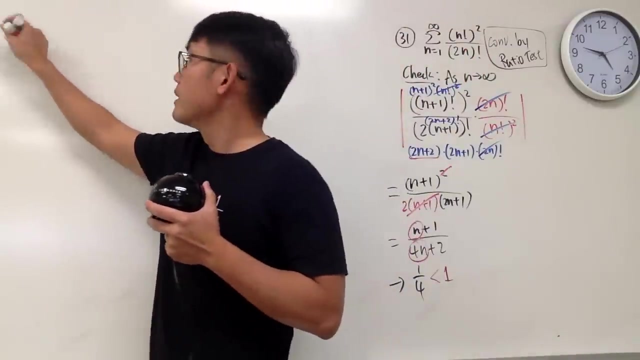 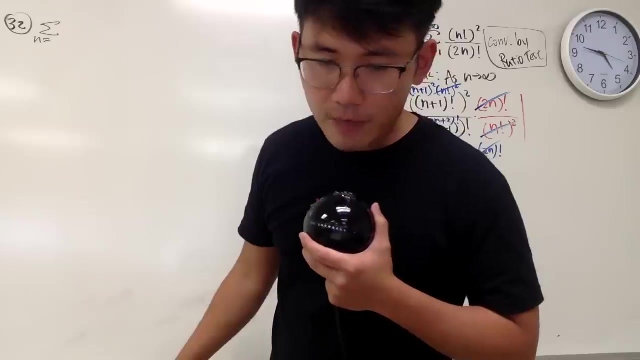 OK. Now OK, Number 32 and number 33,. again, I'm going to do them side by side. I will do them side by side and we'll see how it goes. So we have 1 to infinity And then we have 1 over. 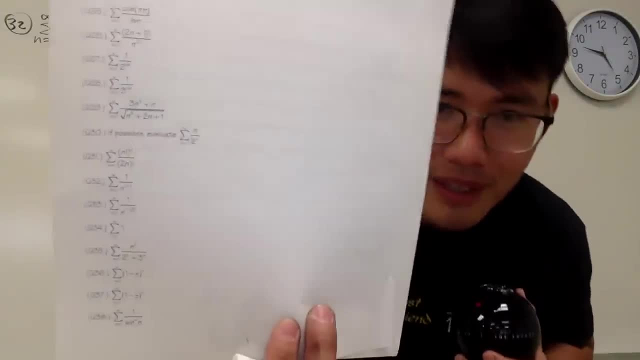 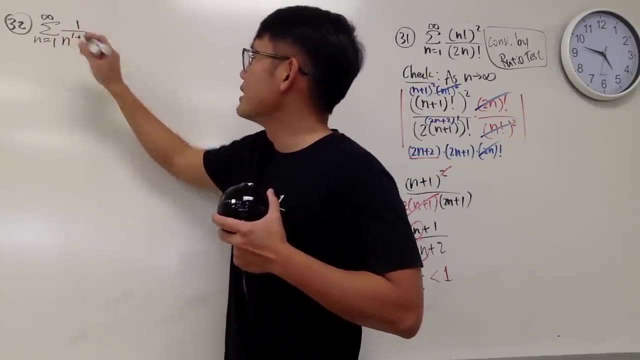 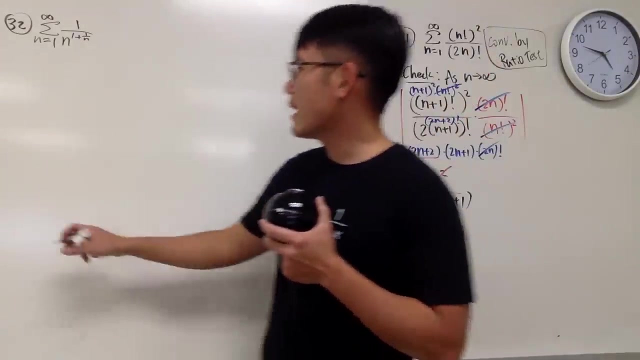 And we have n to the 1 over 1.. n to the 1 plus Oh man, n to the 1 plus 1 over n's power, like that. Hmm, Right, And actually let's just focus on this one first. 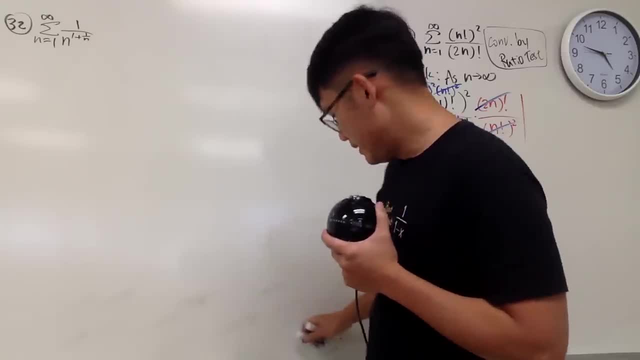 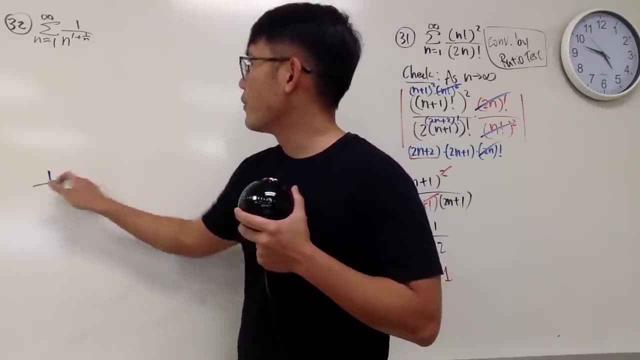 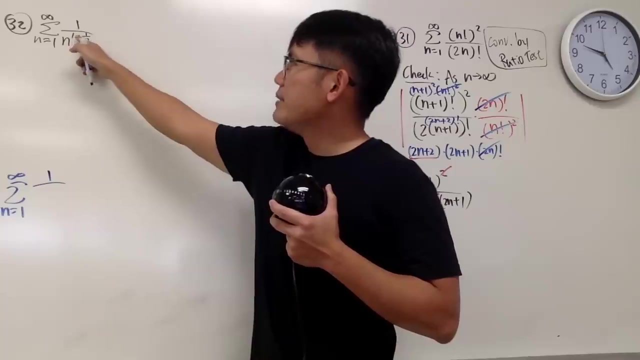 OK, First of all, this is a common mistake for this question. A lot of people will just think that, OK, here we have 1 over the sum, as n goes from 1 to infinity. And OK, we have 1 over n plus 1 over n. 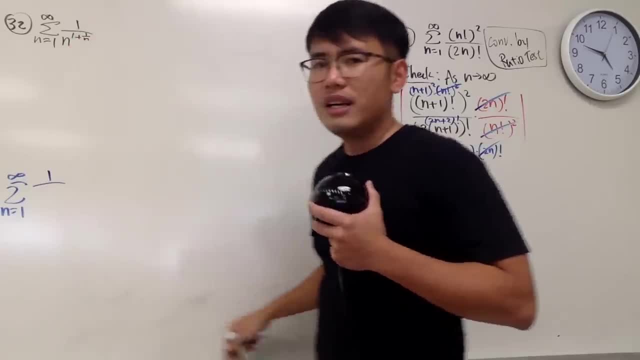 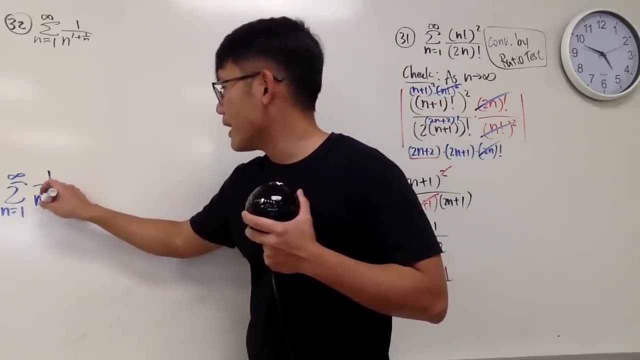 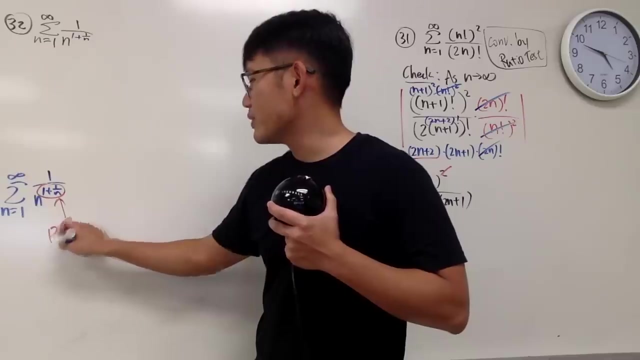 So the numerator, the power, right here it's bigger than 1.. This is a common mistake. You can just, you cannot just do n to the 1 plus 1 over n And say this: right here is the p which is greater, which is this: 1 over 1 plus n. 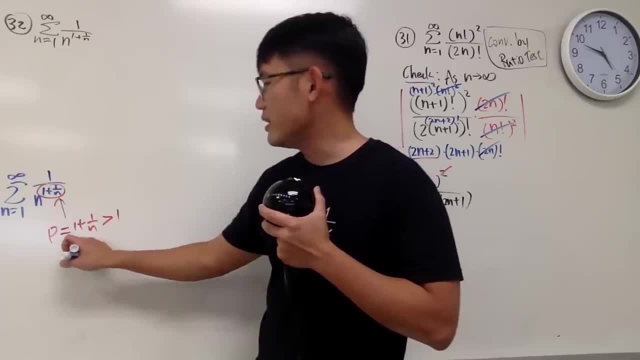 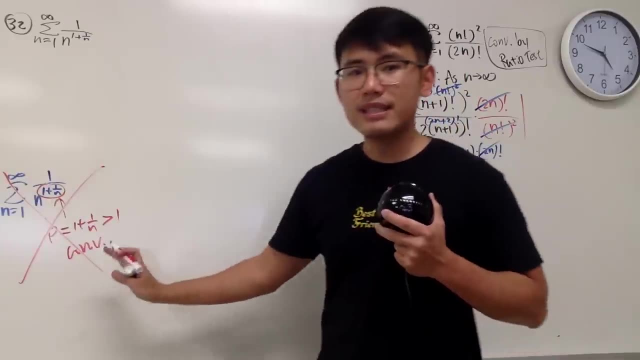 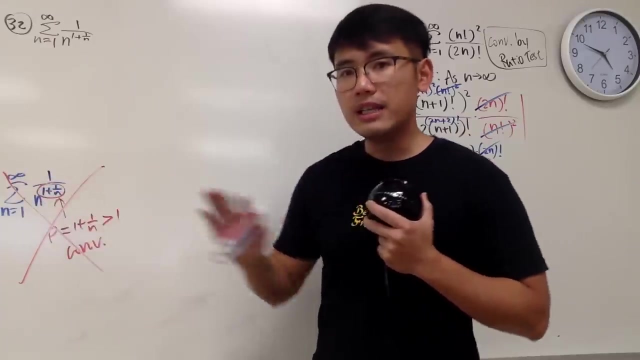 And that's greater than 1.. And you just say it converges. No, A common mistake. No, Cannot do that. Cannot do that. And the reason why is because this 1 over this, 1 plus 1 over n is not a constant, unfortunately. 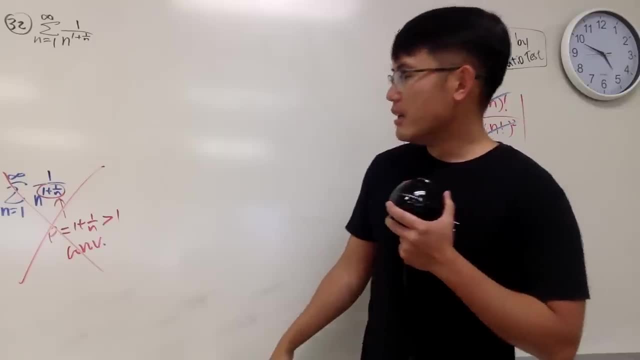 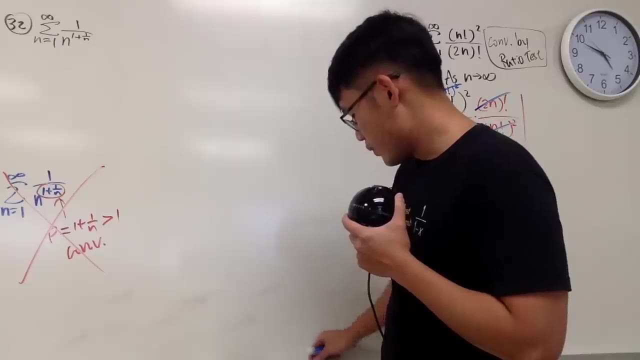 It's not a constant, so we cannot do so, And you really have to just kind of do the comparison test and all that to see what happens. So here we go Right. Here we go First thing. first we have a sum in the power so we can break them apart. 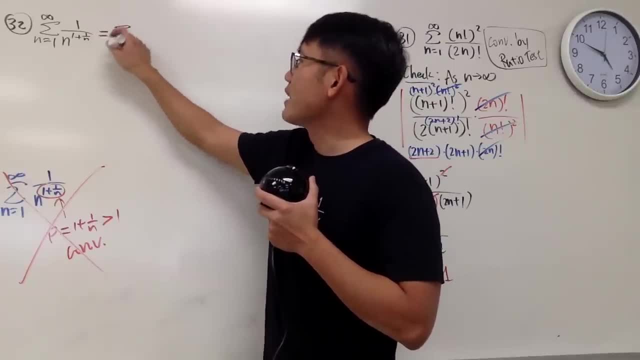 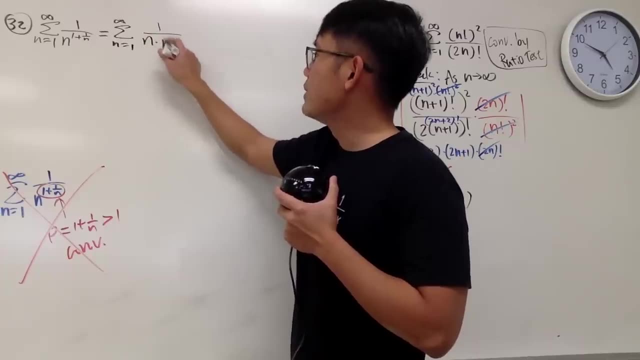 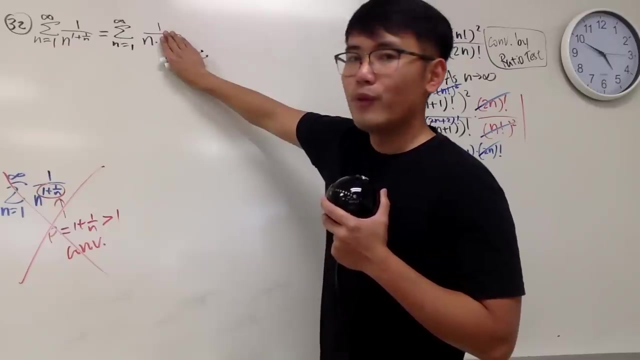 This right here is like saying: we have the sum as n goes from 1 to infinity And we have 1 over n to the first power times, n to the 1 over n power. And I would like to tell you, because we know, the sum of 1 over n diverges. so we'll. 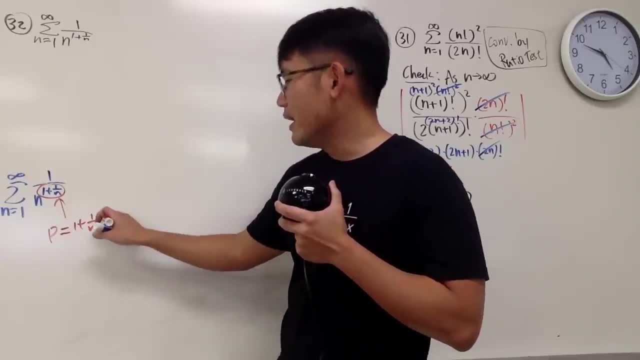 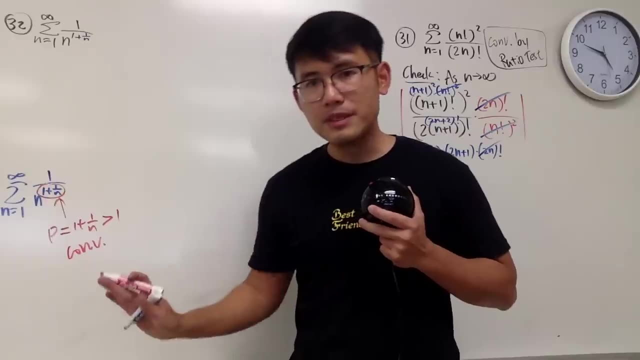 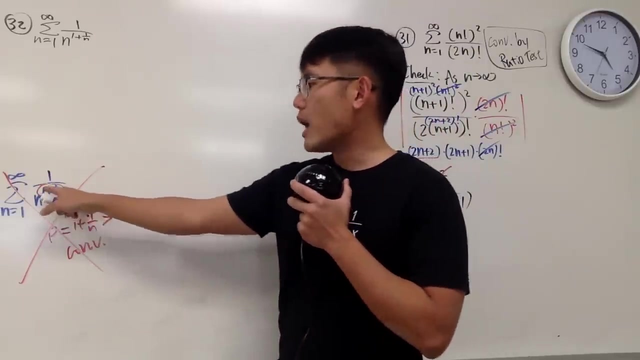 which is this: 1 over 1 plus n, And that's greater than 1.. And you just say it converges. No, A common mistake. No, Cannot do that. Cannot do that. And the reason why is because this 1 over. 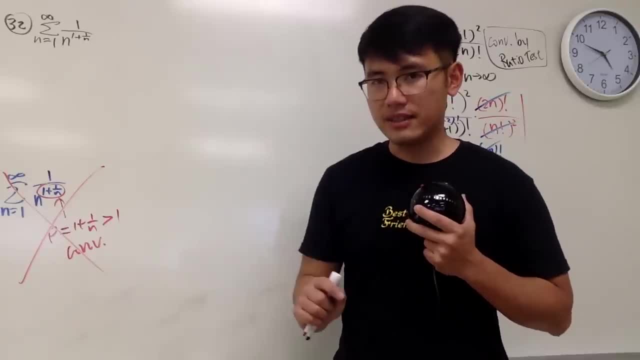 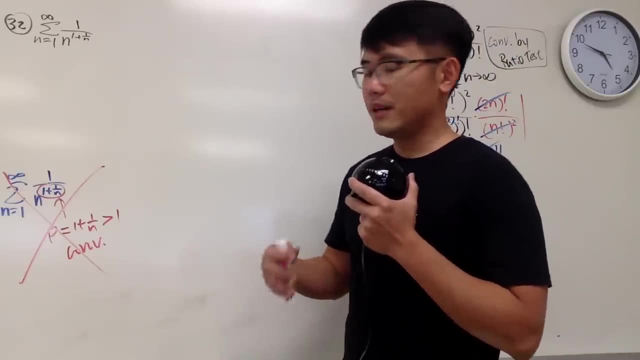 This 1 plus 1 over n is not a constant, unfortunately It's not a constant, so we cannot do so And you really have to just kind of do the comparison test and all that to see what happens. So here we go. 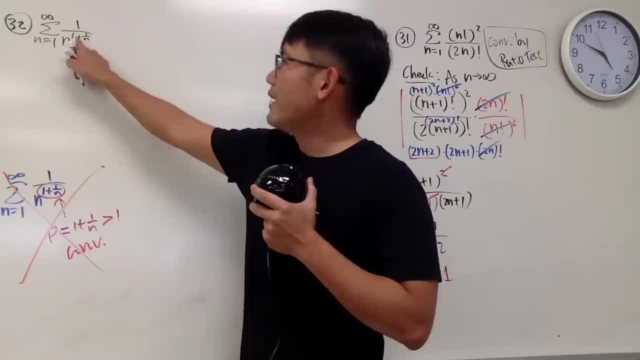 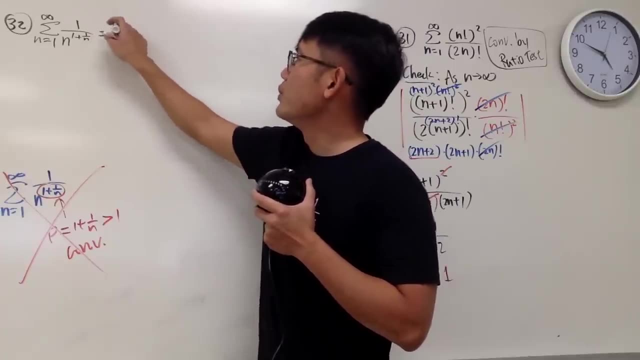 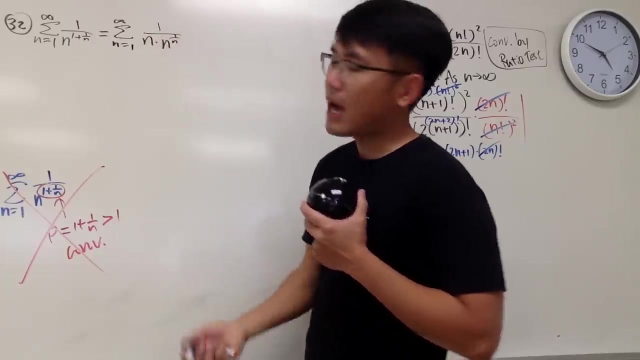 Right Here we go. First thing first, We have a sum in the power so we can break them apart. This right here is like saying: we have the sum as n goes from 1 to infinity, and we have 1 over n to the first power times, n to the 1 over n's power. 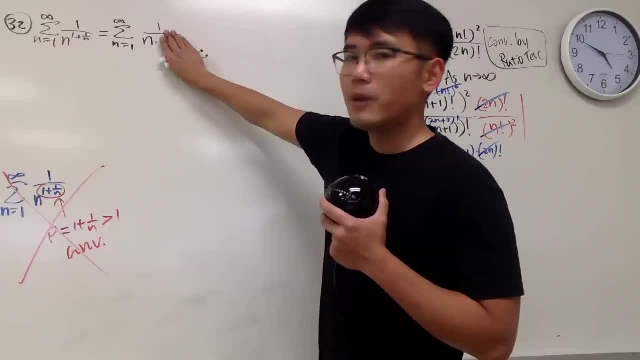 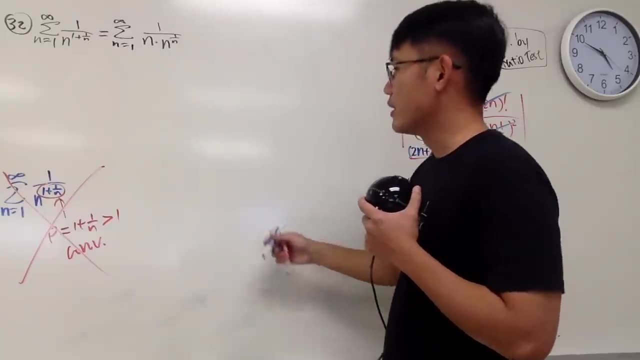 And I would like to tell you, because we know the sum of 1 over n diverges, so we'll actually use that to compute it. And the truth is, I will also write this down right here. I'll just make another note. 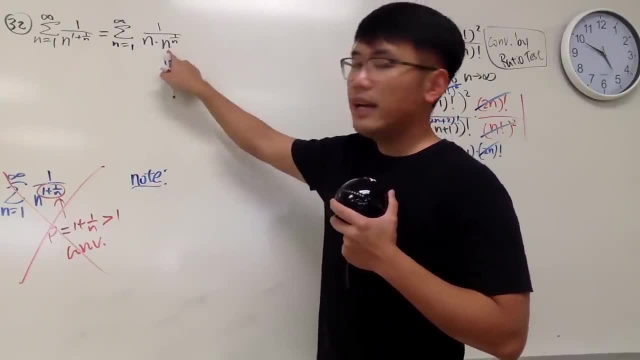 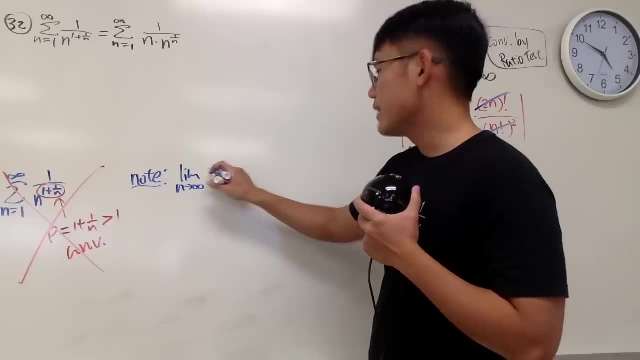 Right. Make another note: If you look at n to the 1 over n, if you take the limit of, n goes to infinity of the, Technically it's just n to the root of n, which is the limit, as n goes to infinity, of n to the 1 over n. 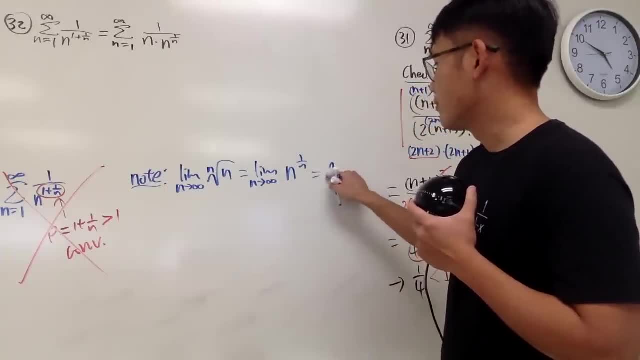 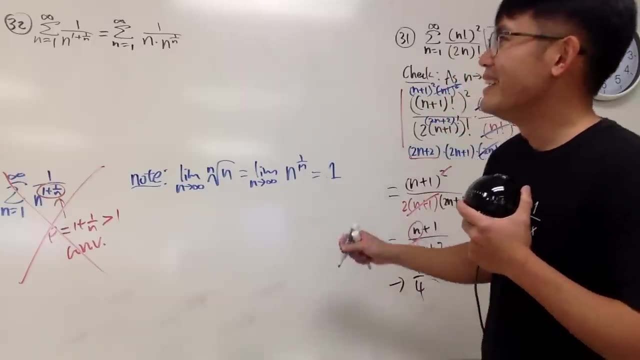 Either way, of course, they are the same thing. This right here, you actually get 1.. Okay, You can check out my other video for the limit right here, or you can just try it on your own. up to you. 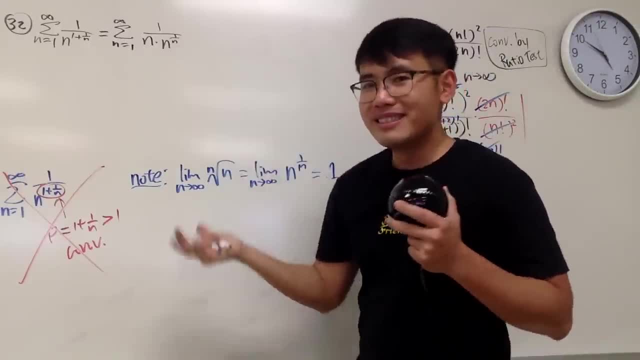 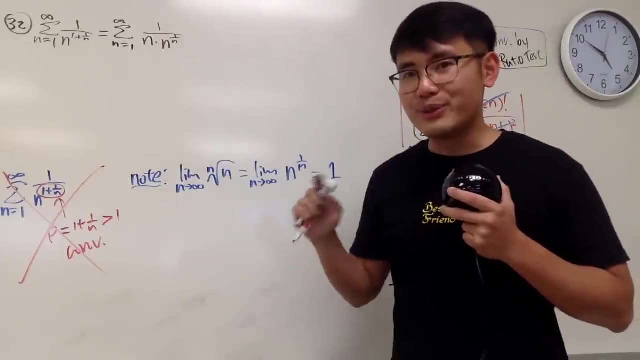 So this right here it doesn't have any like say, because it's not approaching infinity whatsoever or it's causing 0 whatsoever. So I will use 1 over n, the series, for that to make our comparison. So here we go. 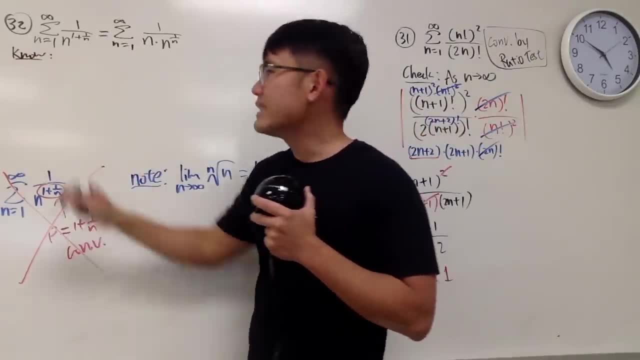 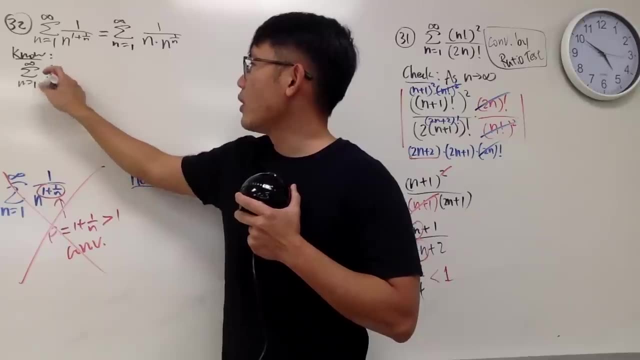 Let me just put down what we know. We know that the sum as n goes from 1 to infinity, 1 over n. right here again, this is to the first power. so I will put down: p is equal to 1,. 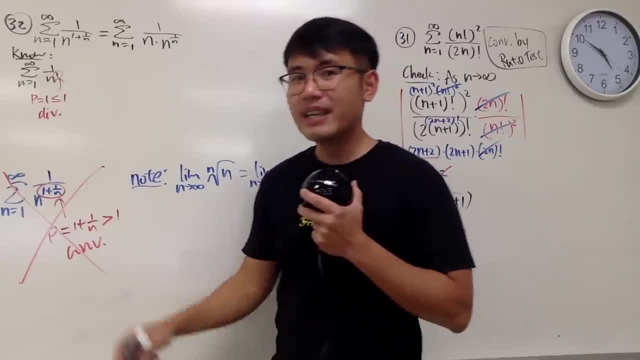 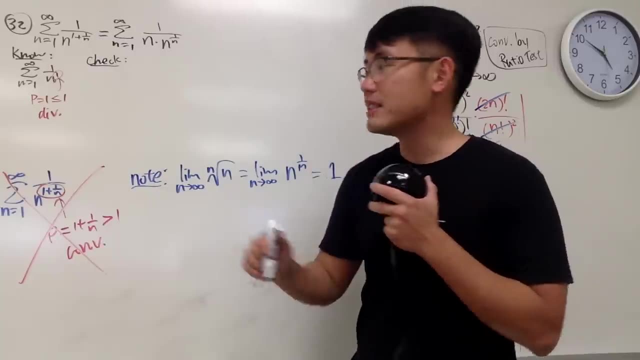 which is less than or equal to 1, which, right here, diverges. Now we are going to do the check And what we are going to do is the limit comparison test. You will see, this is actually the same size as that, about the same size. 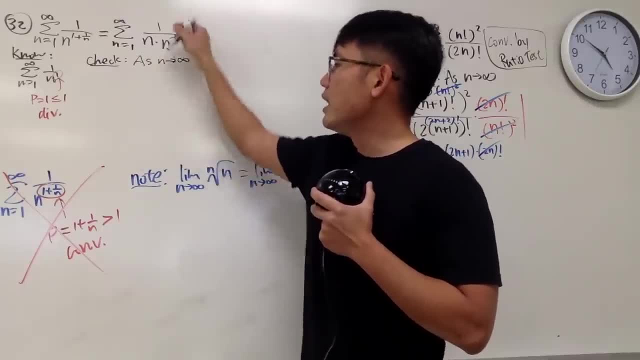 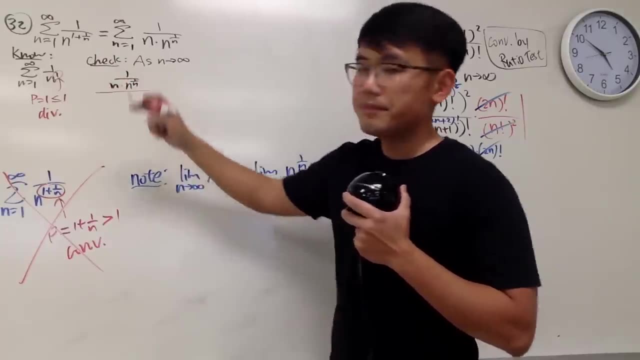 Right. So as n goes to infinity, I will put this 1 on the top like this: n times n to the 1 over n power, and then we'll divide it by 1 over n. right here Do the algebra Take this flip that. 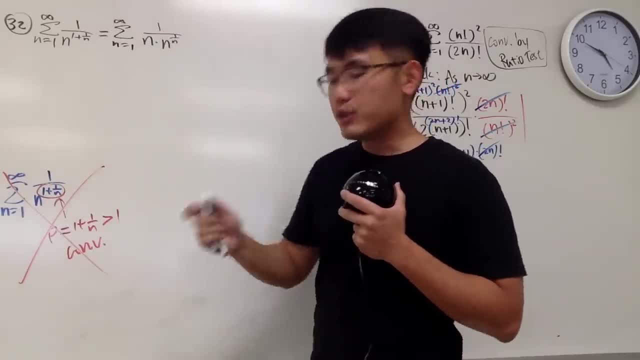 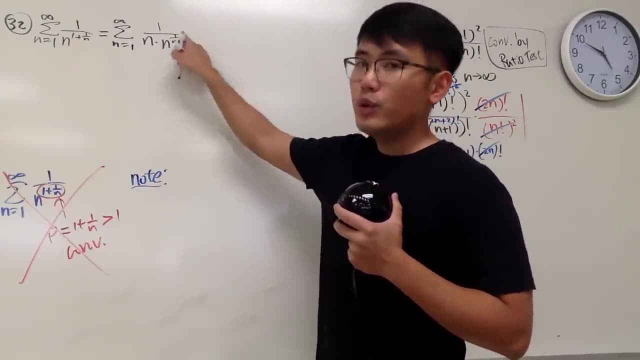 actually use that to compute it. And the truth is I will also write this down right here. I'll just make another note. Right, Make another note. If you look at n to the 1 over n, if you take the limit of n goes to infinity of the technically 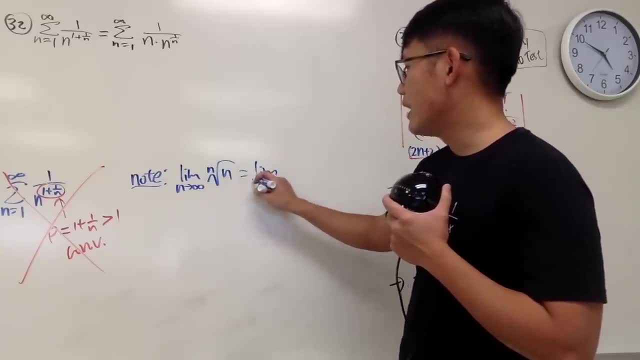 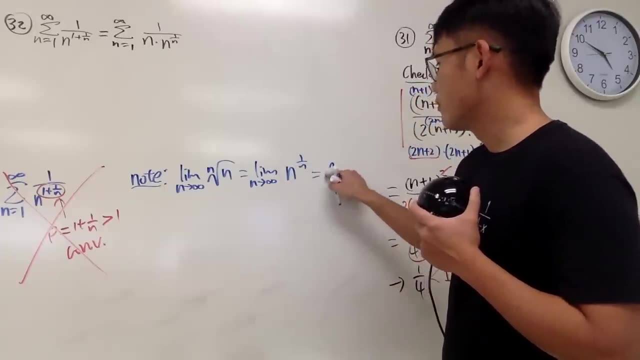 it's just n to the root of n, which is the limit, as n goes to infinity, of n to the 1 over n. Either way, of course, they are the same thing. This right here, you actually get 1.. Okay. 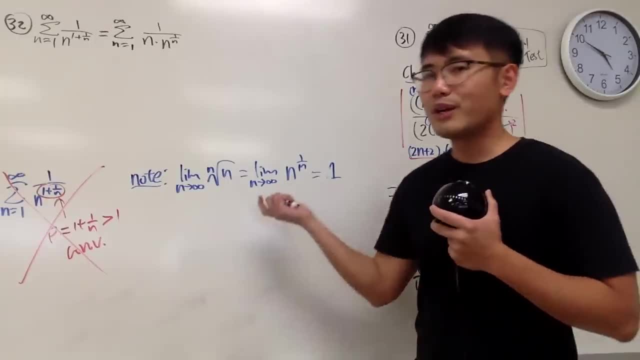 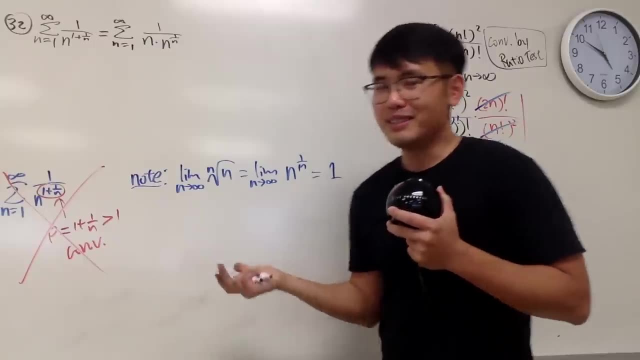 You can check out my other video for the limit right here, or you can just try it on your own, Up to you. So this right here it doesn't have any say because it's not approaching infinity whatsoever or it's causing 0 whatsoever. 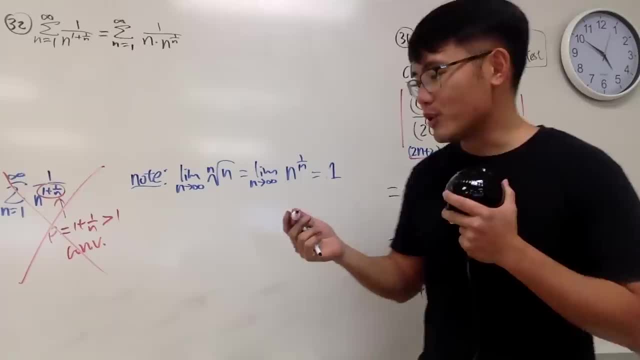 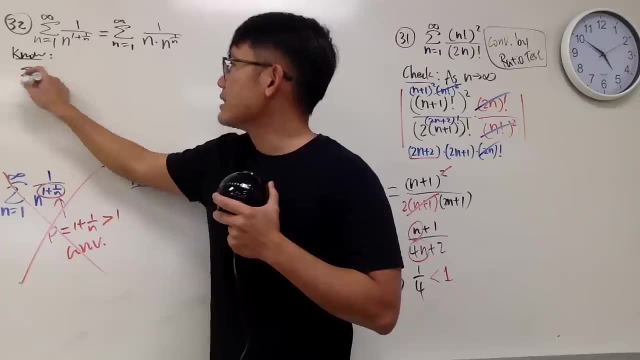 So I will use 1 over n, the series, for that to make our comparison. So here we go. Let me just put down what we know. We know that the sum as n goes from 1 to infinity: 1 over n, right here. 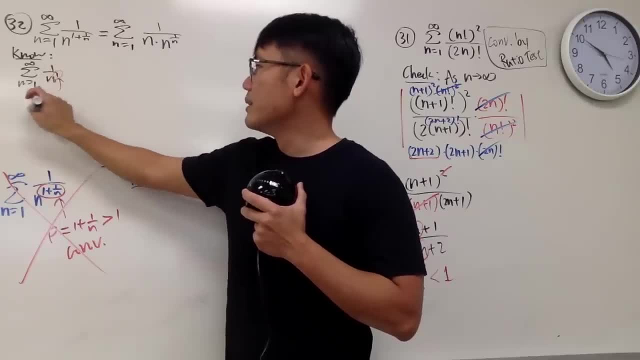 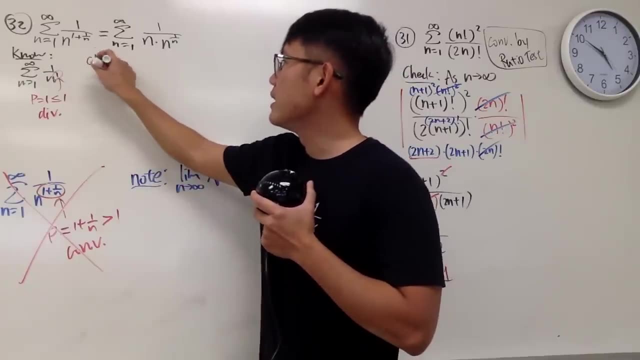 Again, this is to the first power. So I will put down: p is equal to 1,, which is less than or equal to 1, which right here diverges. Now we are going to do the check And what we are going to do is the limit comparison test. 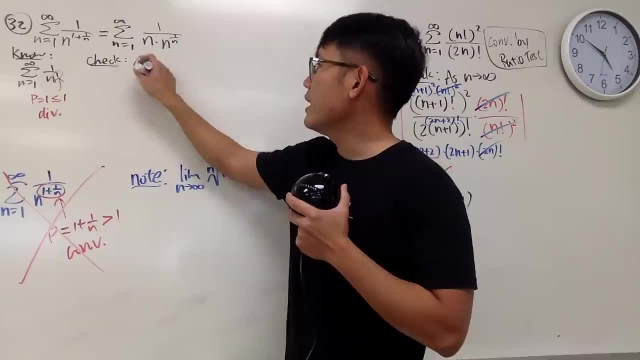 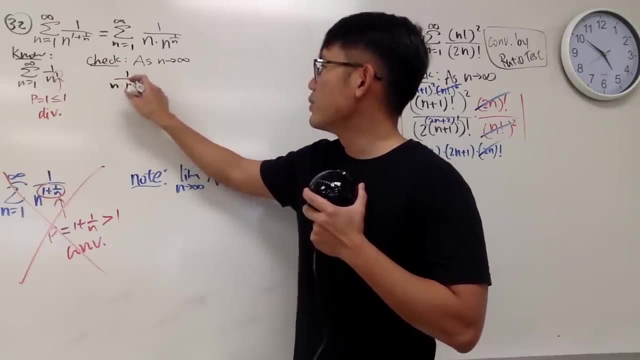 You will see, this is actually the same size as that. about the same size, Right? So I'll say, as n goes to infinity, I will put this one on the top like this: n times n to the 1 over n power. 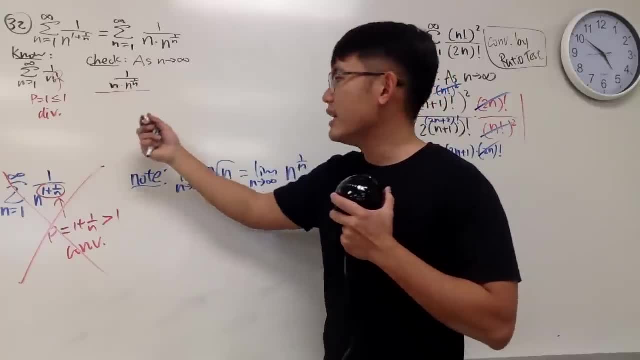 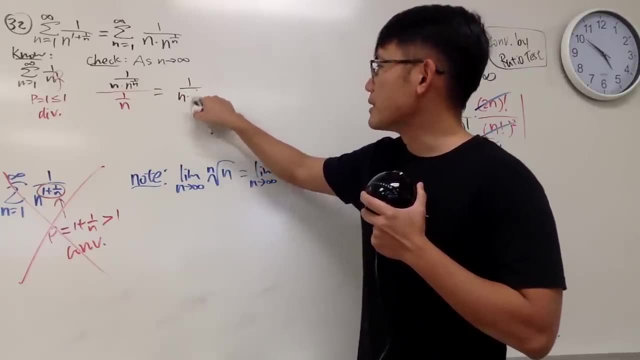 And then we'll divide it by 1 over n. right here Do the algebra. Take this flip that We get 1 over n times 1 times n to the 1 over n power, And take the reciprocal, which is n over 1.. 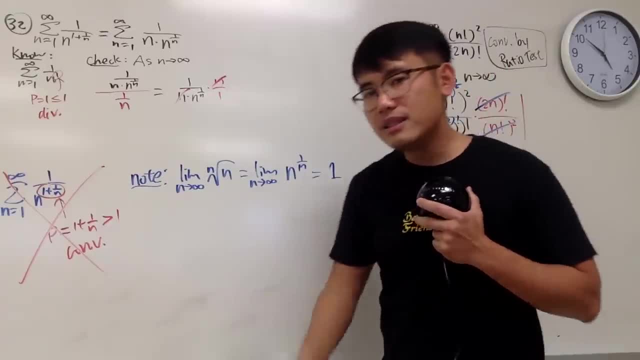 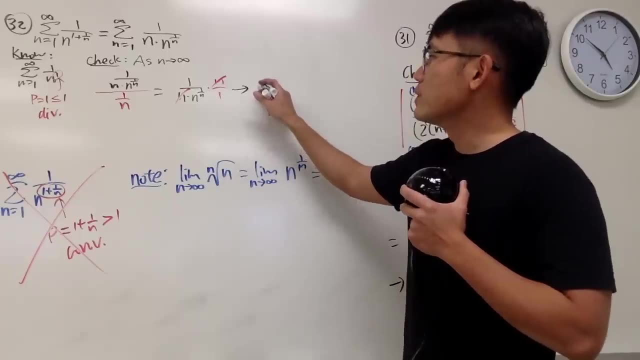 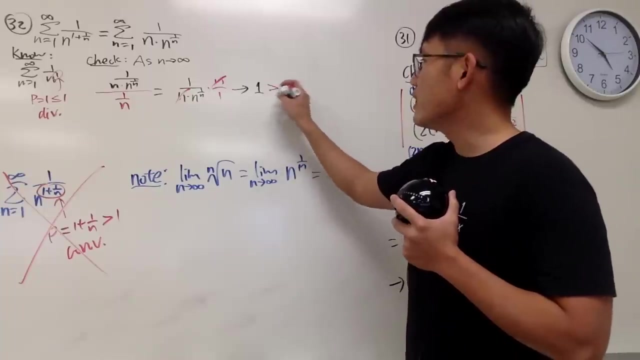 And you see this and that will cancel And you see that this right here is actually approaching 1.. So you see 1 over 1, pretty much This right here approaches 1.. And we are doing the limit comparison test. 1 is useful and we have to say 1 is greater than 0. 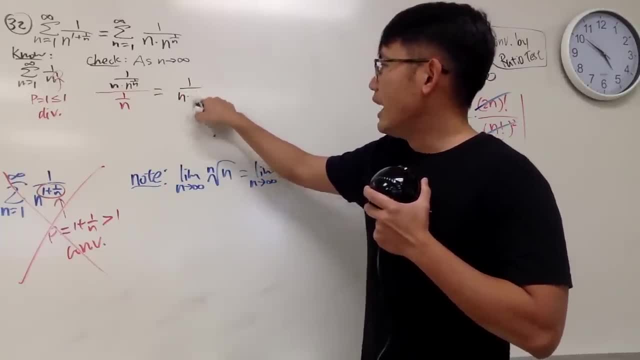 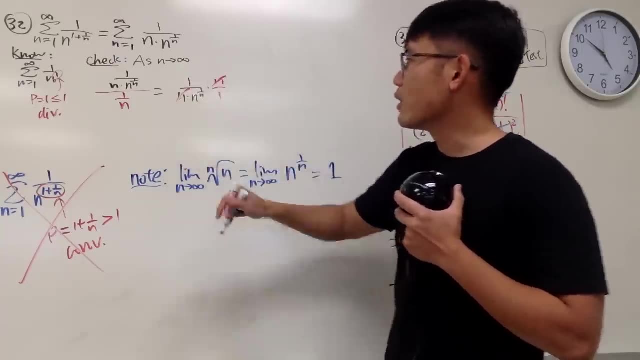 We get 1 over n times 1 times n to the 1 over n power. and take the reciprocal, which is n over 1, and you see this and that will cancel, And you see that this right here is actually approaching 1.. 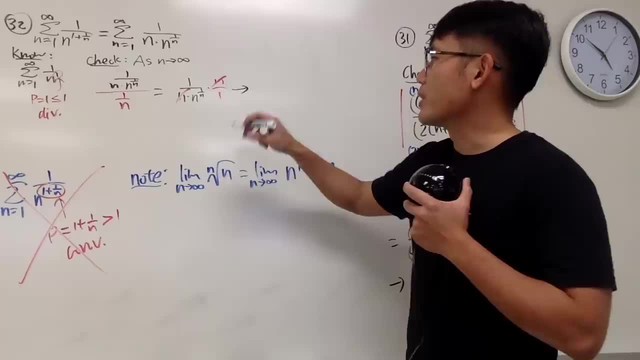 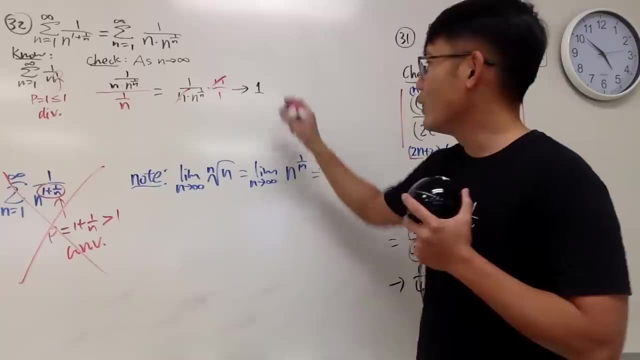 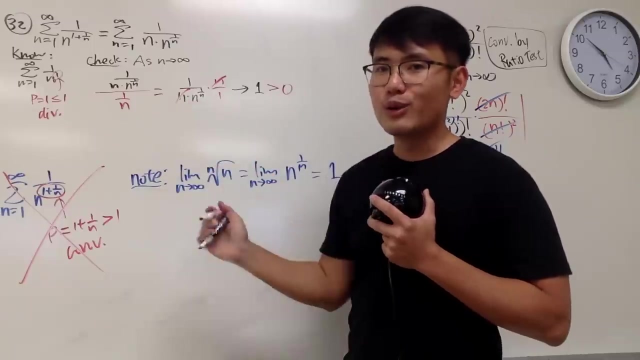 So you see 1 over 1, pretty much This right here approaches 1. And we are doing the limit comparison test. 1 is useful and we have to say 1 is greater than 0. So in another word, they are about the same size, as n goes to infinity. 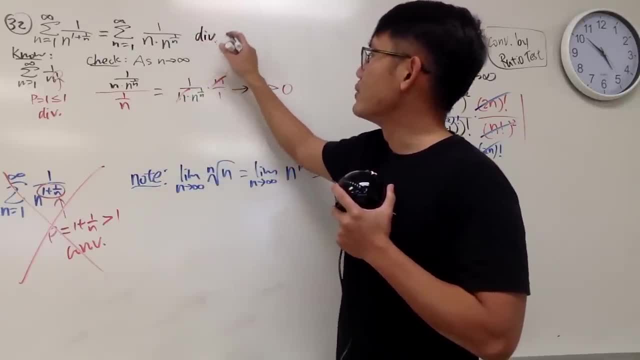 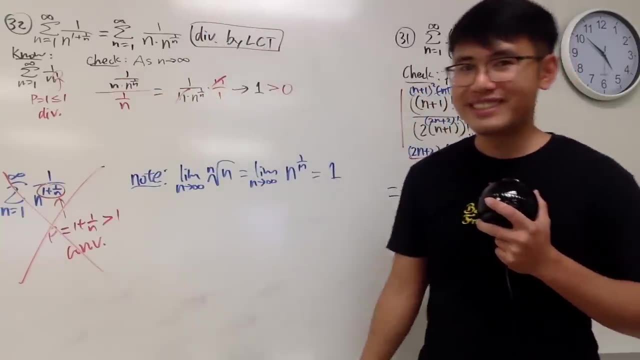 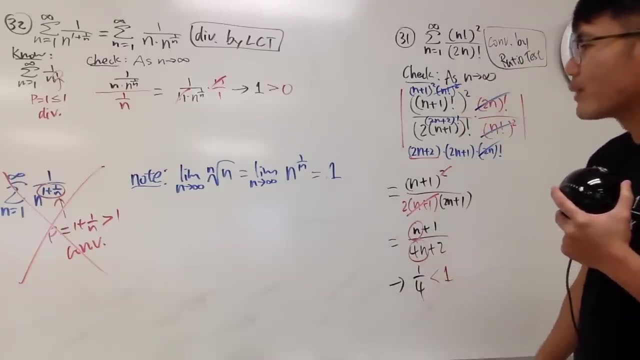 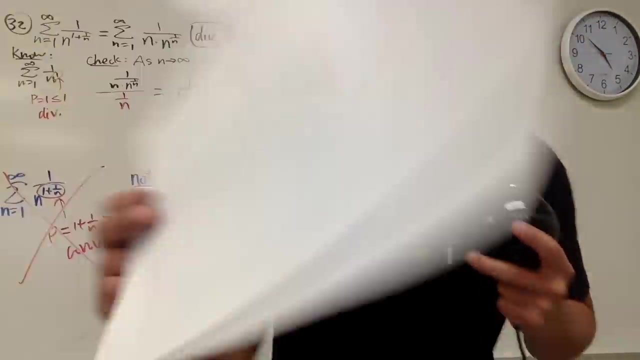 So in another word, this right here also diverges by the limit comparison test with the harmonic series. on that, All right. So that's pretty much the idea. Okay, Now we are going to do. I just made the 1 over n become 1 over n squared. 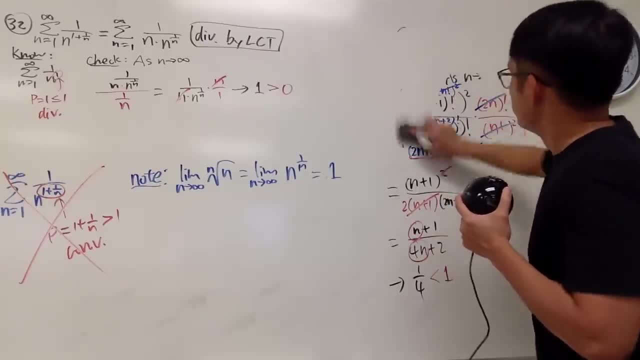 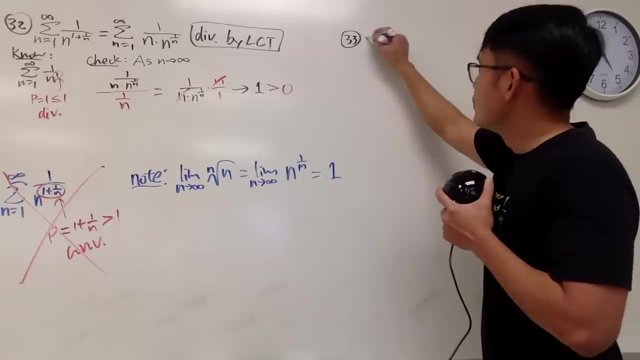 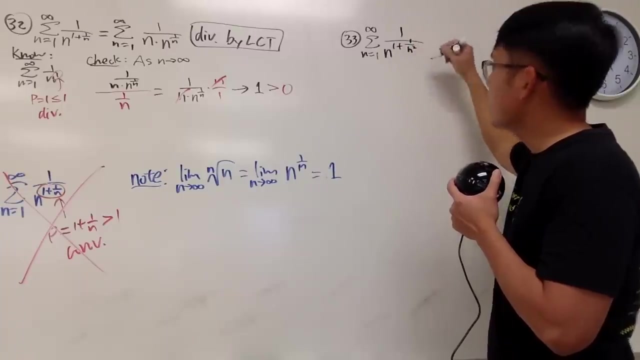 So let's see what will happen, right? So number 33.. We are going to do the sum as n goes from 1 to infinity, and this is 1 over n to the 1 plus 1 over n squared, And of course we can do that. 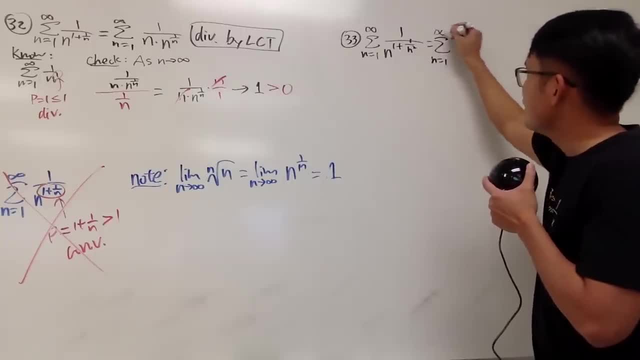 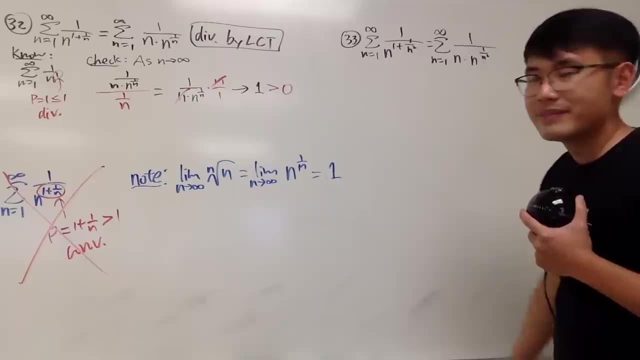 So this is the same as saying the sum as n goes from 1 to infinity, of 1 over n to the first power times, n to the 1 over n squared power, Same thing. And again, if you are doing this from scratch, 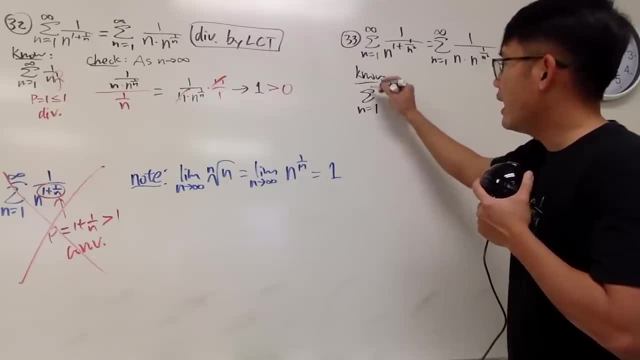 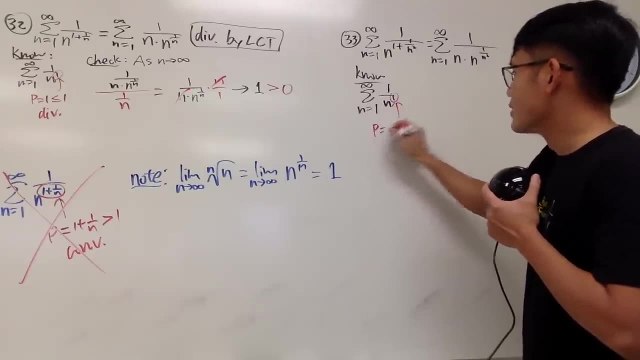 I will just write this down again for you guys. We have to know that the series as n goes from 1 to infinity, of 1 over n to the first power, the harmonic series diverges. so p is 1,, which is less than or equal to 1,. 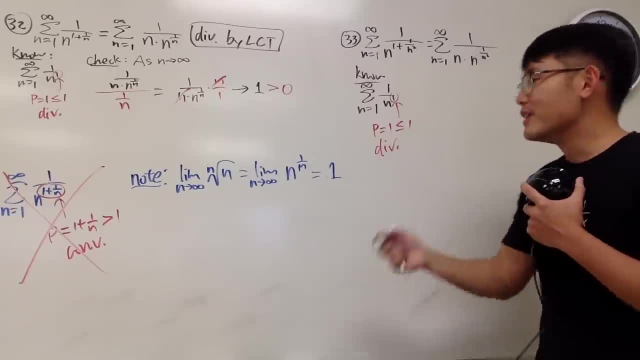 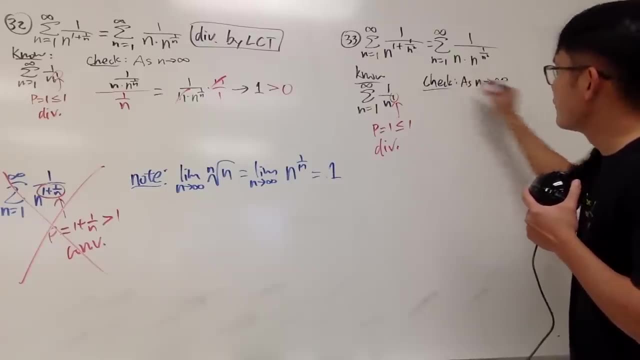 and this right here diverges. right Now, check, Here is the deal. We will just say: check as n goes to infinity. Well, I will put this on the top, which is 1 over n times n to the 1 over n squared power. 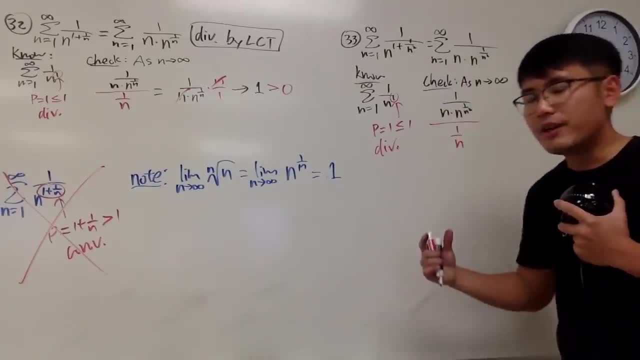 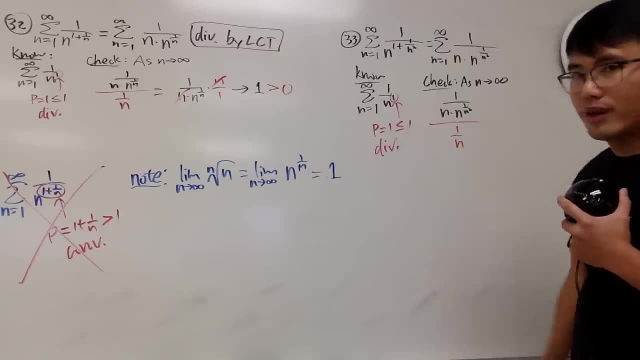 and then divide it by 1 over n. This right here the say is the 1 over n to the first power. It has the dominating part. Do not use 1 over n squared right. Do not use 1 over n squared. 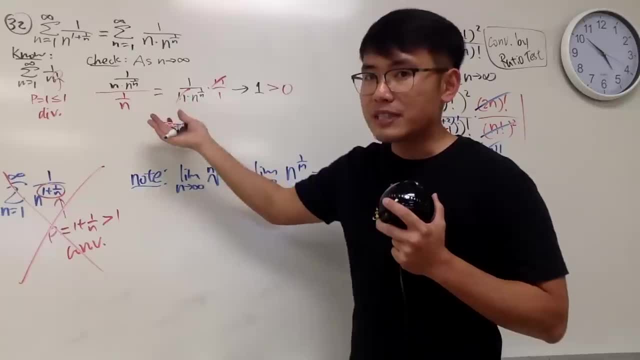 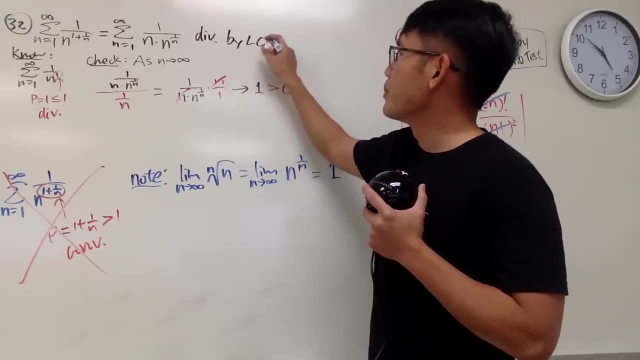 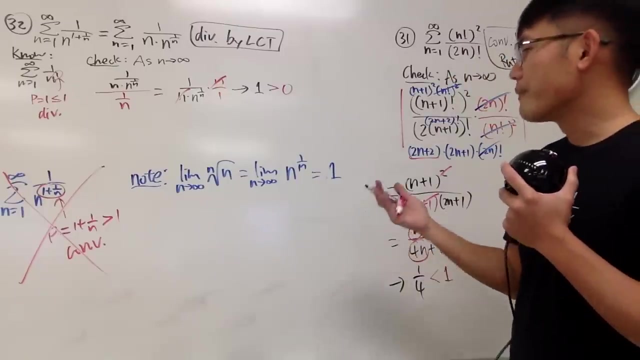 So in another word, they are about the same size as n goes to infinity. So in another word, this right here also diverges by the limit comparison test with the harmonic series. on that, All right. So that's pretty much the idea. 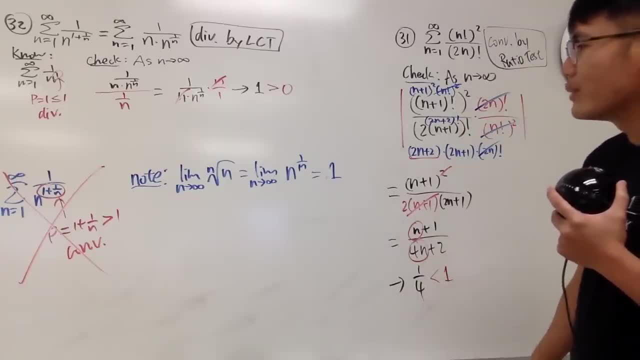 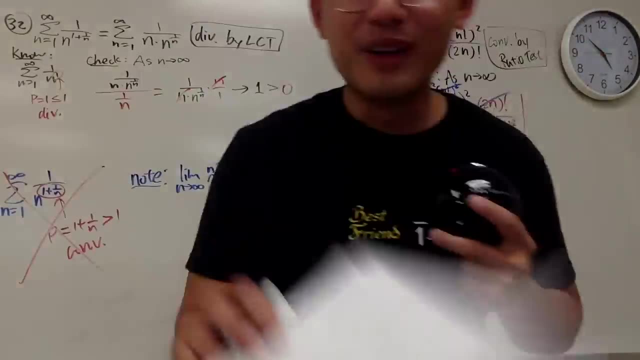 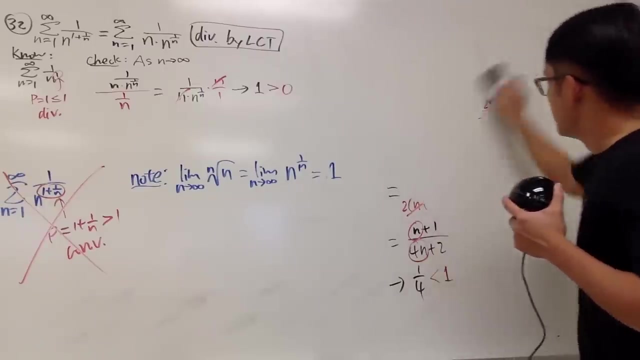 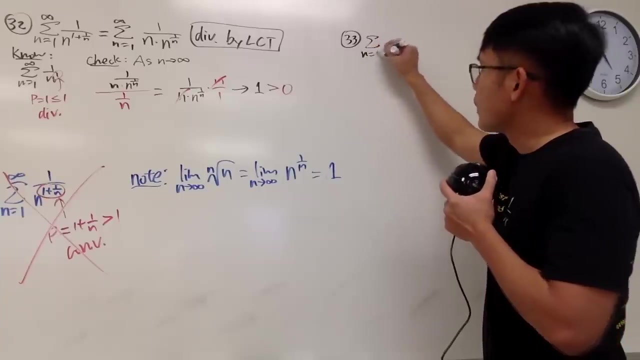 OK, Now we are going to do well, just make the 1 over n become 1 over n squared. So let's see what will happen, right? So number 33.. We are going to do the sum as n goes from 1 to infinity. 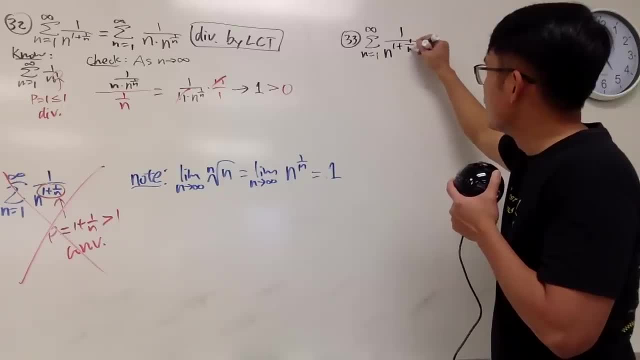 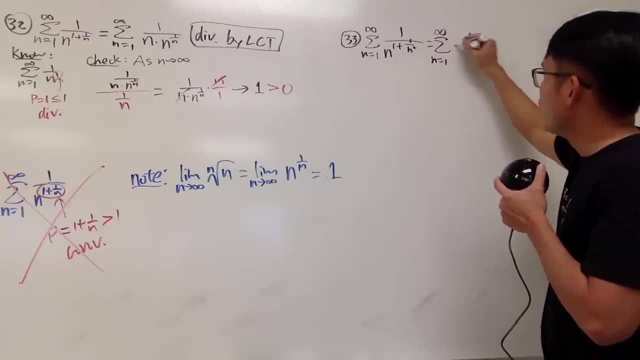 And this is 1 over n to the 1 plus 1 over n squared, And of course we can do that. So this is the same as saying the sum, as n goes from 1 to infinity, of 1 over n to the first power times, n to the 1 over n squared power. 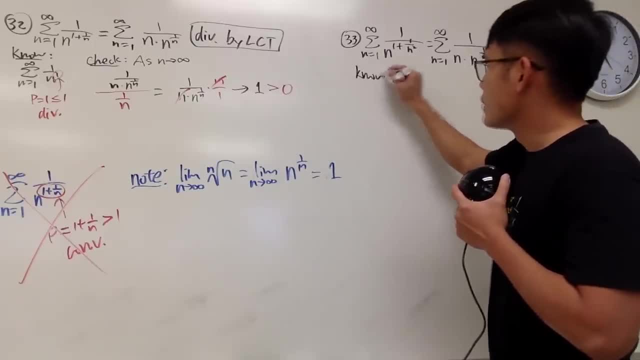 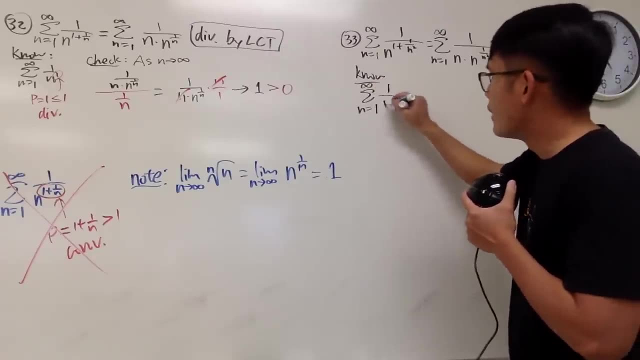 Same thing. And again, if you are doing this from scratch, I will just write this down again for you guys. We have to know that the series as n goes from 1 to infinity of 1 over n to the first power, the harmonic series diverges. 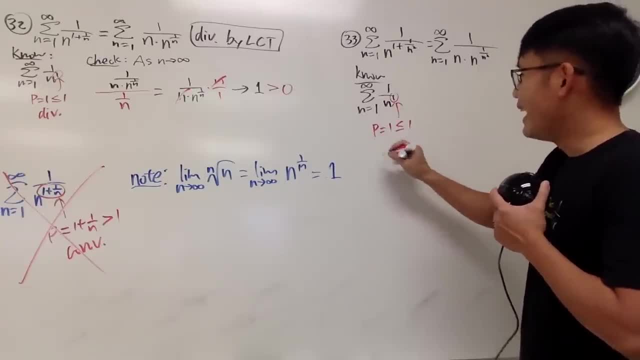 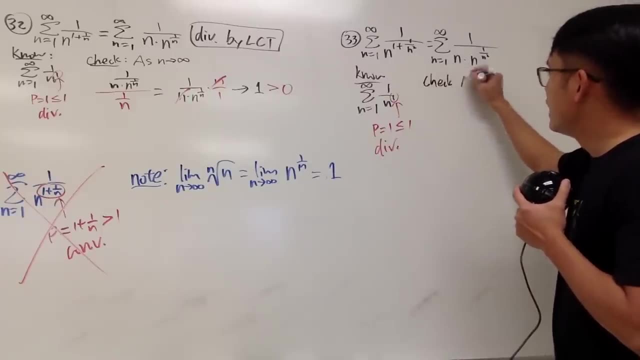 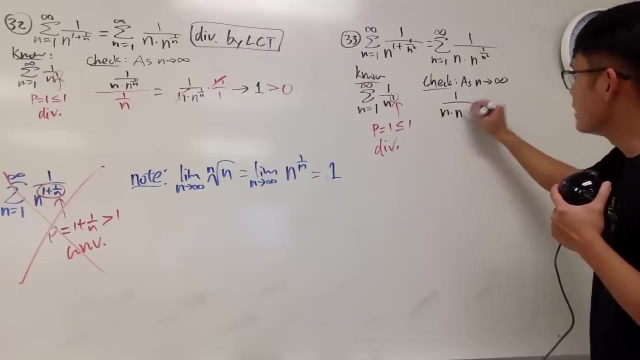 So p is 1, which is less than or equal to 1.. And this, right here, diverges. Right Now, check. Here is the deal. We will just say check as n goes to infinity. Well, I will put this on the top, which is 1 over n times n to the 1 over n squared power. 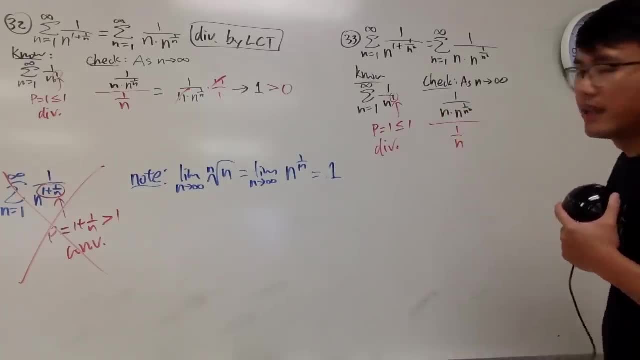 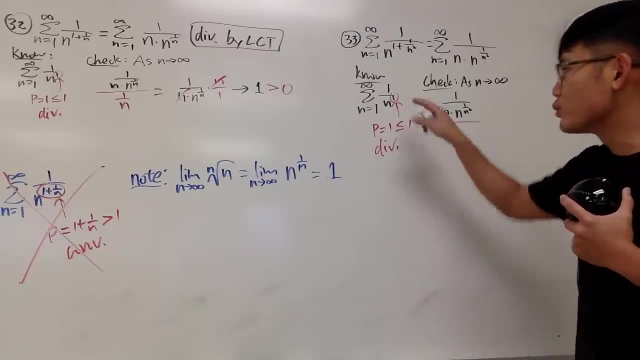 And then divide it by 1 over n. This, right here, let's say, is the 1 over n to the first power. It has a dominating part. Do not use 1 over n squared Right. Do not use 1 over n squared. 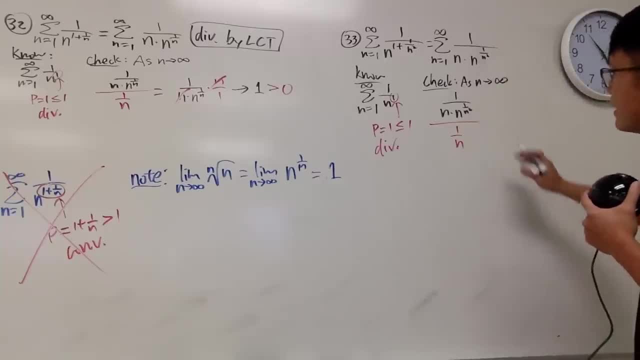 Even though you see the 1 over n squared here as 1 over n squared. OK, This is the deal, But don't do that. So here is the deal. Flip that as the probability over there. So 1 over n times 1 over n squared times n over 1.. 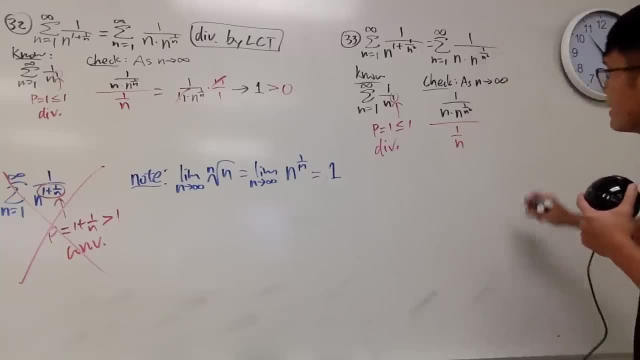 even though you see the 1 over n squared here as well. but don't do that. So here is the deal. Flip that as the probability over there. so 1 over n times n to the 1 over n squared times n to the 1 over 1,. 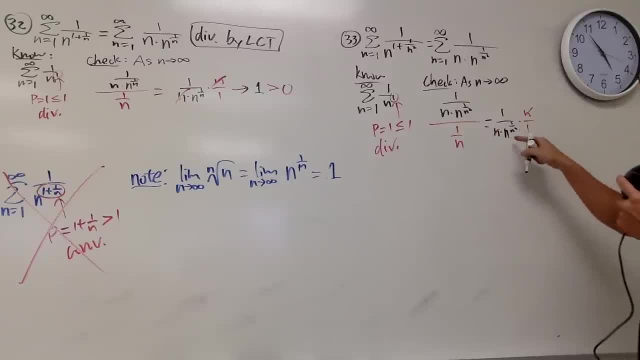 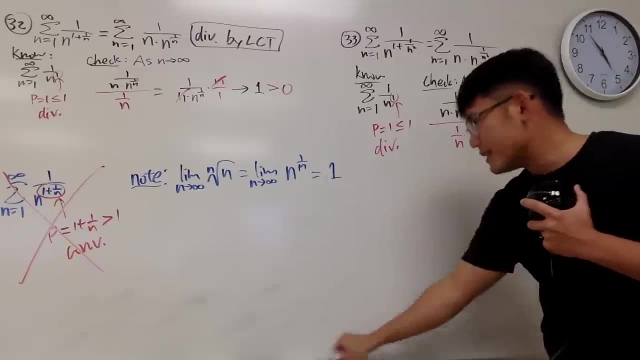 cancel, cancel and we end up with this, which is a very, very similar situation. So I didn't show you guys the work over there. I will show you guys the work here now, so let's see what happens with that, okay. 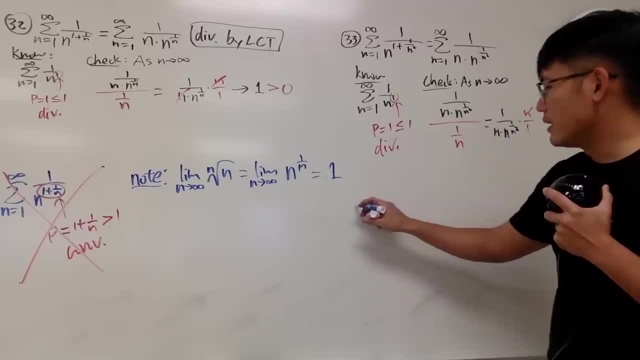 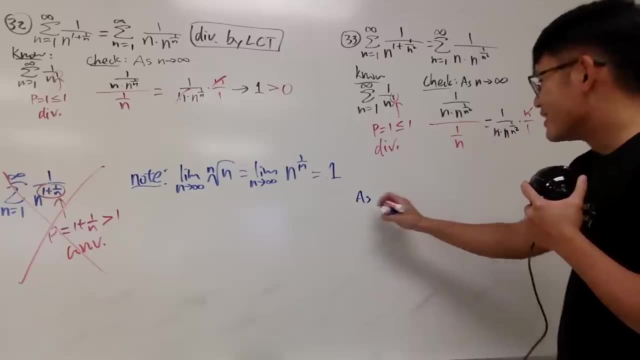 So I will just tell you guys, let's do x right, So let's put down x. So I will just say x, because I will use Lapito's rule, so I have to use derivative, So as x goes to infinity. 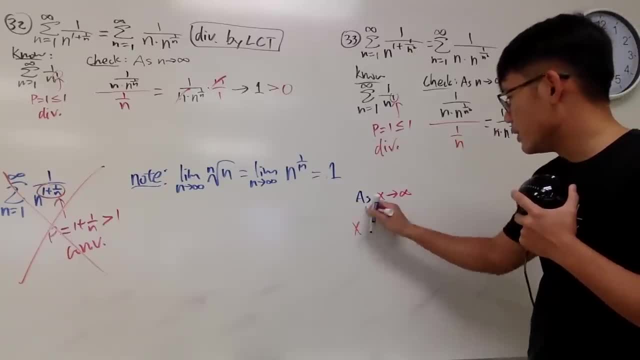 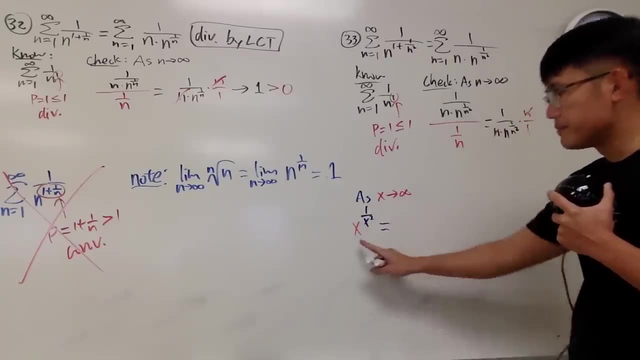 right. So we have x to the 1 over x power like this: 1 over x squared power. This is how you do it: x is the same as e to the ln x power, and then you can take this and raise that to the 1 over x squared power. 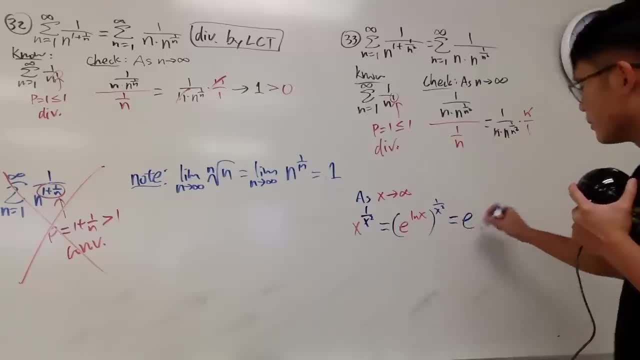 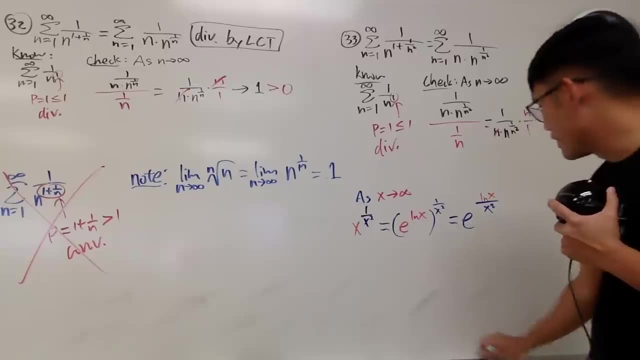 Okay, So here we have e, and then, of course, you just kind of multiply the powers, you get ln x over x squared and you focus on the derivatives right here and you want to take: well, this is Lapito's rule already. 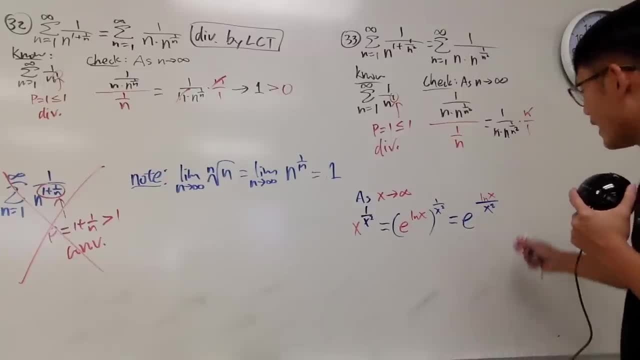 so you can see. well, in fact you don't even need to use Lapito's rule. Why? Because you see that this right here is from the list, so you could have just used n. But anyway, this right here goes to 0,. 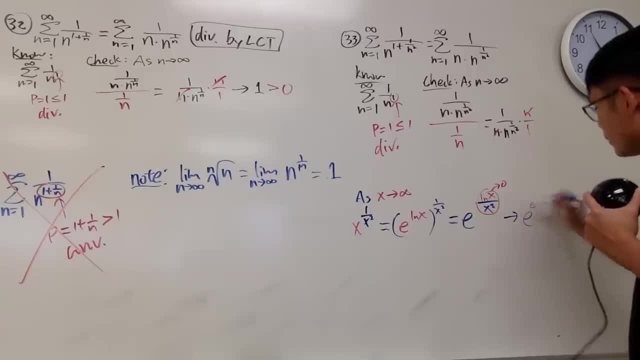 so it pretty much goes to e, to the 0, which is another, just 1.. So this right here also gives you 1 as well. It also goes into 1.. And this right here is greater than 0, so same speech, right. 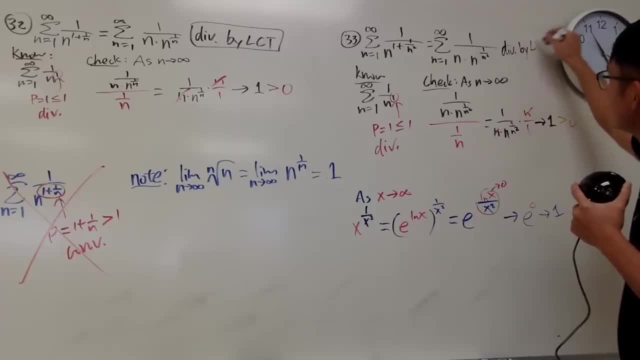 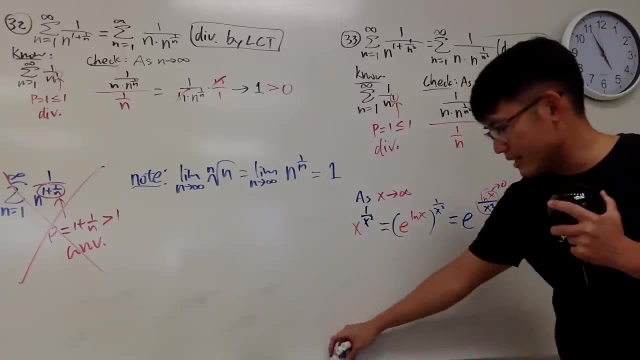 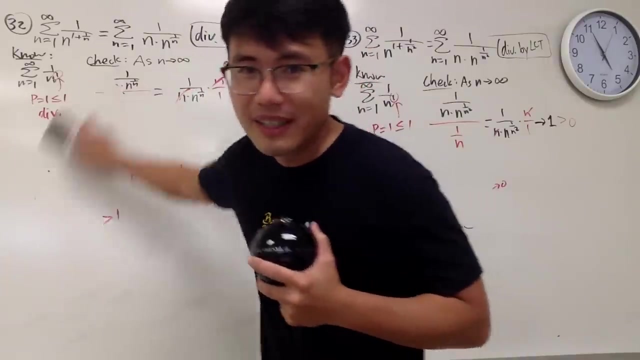 This right here diverges by the ln, and then we are done. right, So that is the idea, Right, Cool. So now we did a lot of questions. How much time is this? 2 hours and 30 minutes. 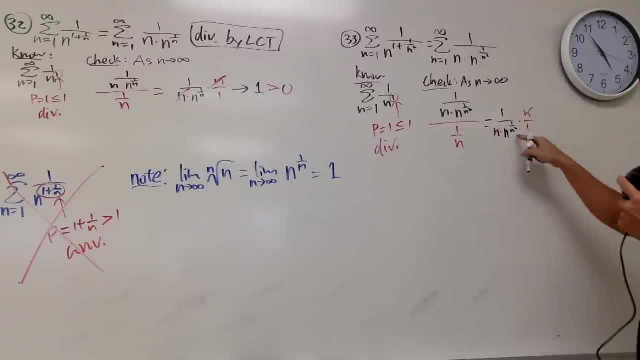 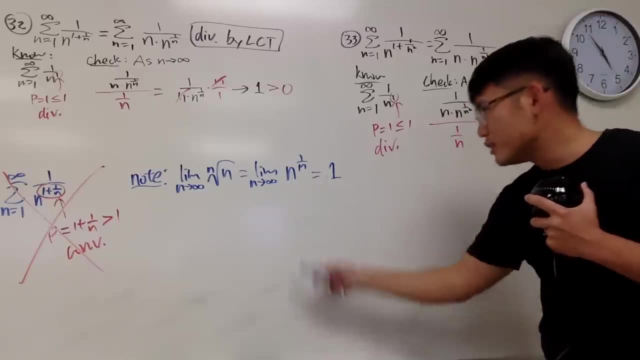 Cancel, cancel And we end up with this, which is a very, very similar situation. So I didn't show you guys the work over there. I will show you guys the work here now. So let's see what happens with that. 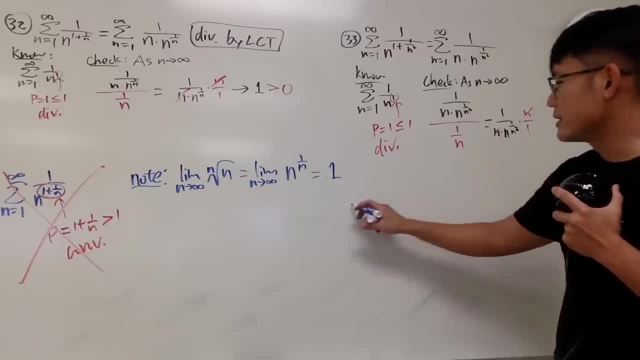 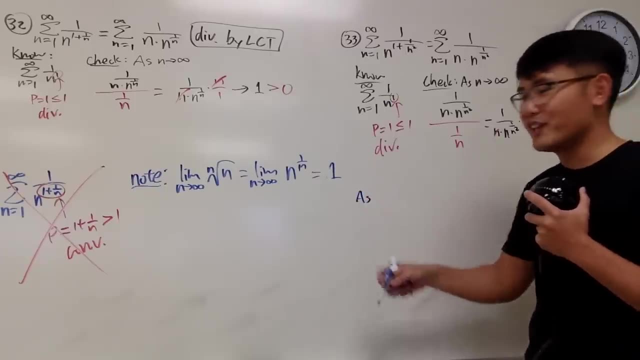 OK. So I will just tell you guys, Let's do x, Right, So let's put down x. So I will just say x, Because I will use Lapito's rule, so I have to use derivative, So as x goes to infinity. 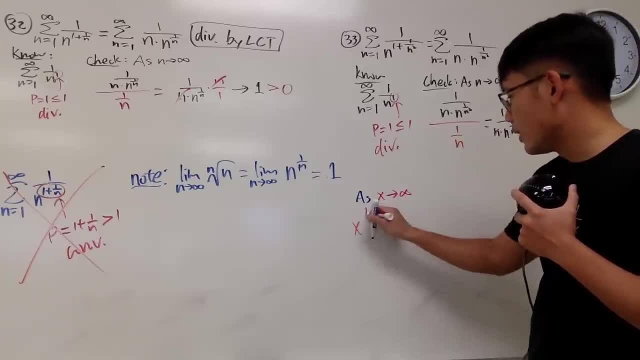 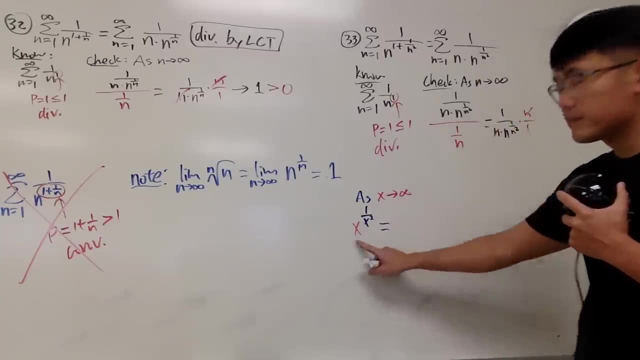 Right, So we have x to the 1 over x power like this: 1 over x squared power. This is how you do it: x is the same as e to the ln x power And you can take this and raise that to the 1 over x squared power. 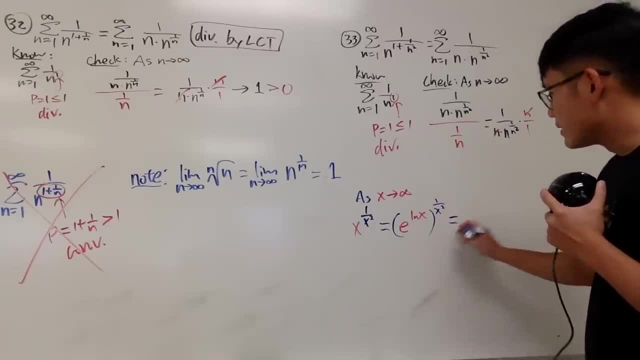 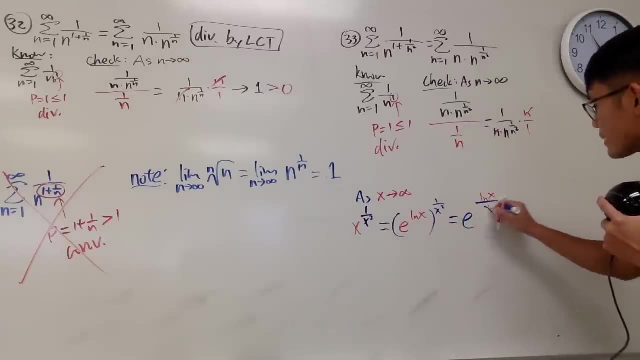 OK, So here we have e, And then of course, you just kind of multiply the powers. You get ln over x squared, And then you focus on the derivatives right here And you want to take: Well, this is Lapito's rule already, so you can see. 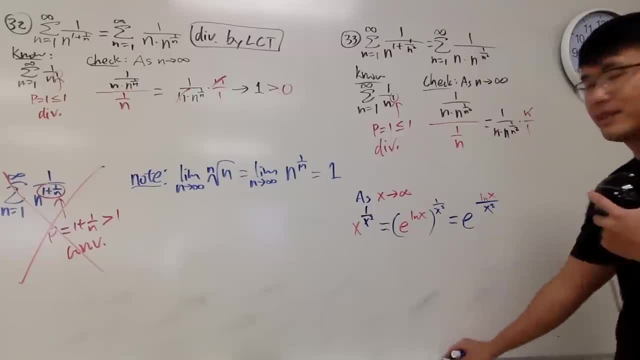 Well, in fact, you don't even need to use Lapito's rule. Why? Because you see that this right here is from the list, So you could have just used n, But anyway, this right here goes to 0.. 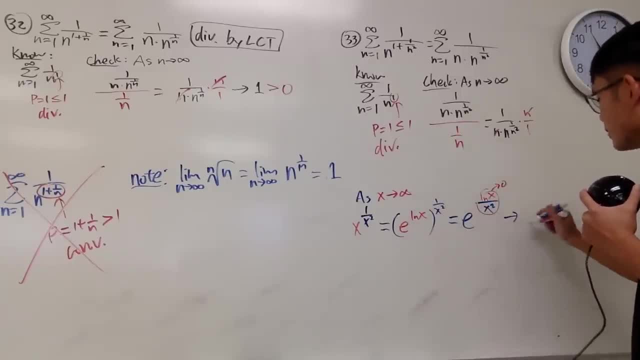 So the derivative is 1 over x squared. This right here goes to 0.. So it pretty much goes to e, to the 0, which is another Just 1.. So this right here also gives you 1 as well. 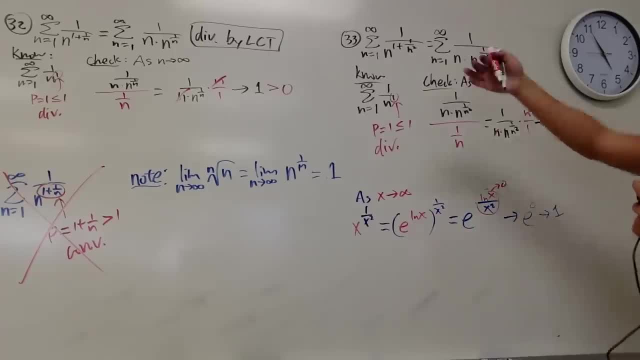 It also goes to 1. And this right here is greater than 0. So same speech, Right. This right here diverges by the lct, And then we are done, Right. So that is the idea, Right. 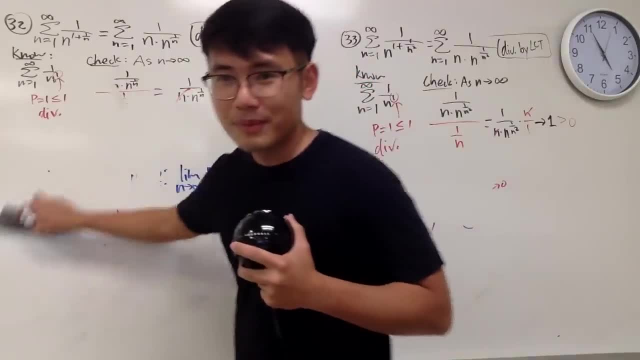 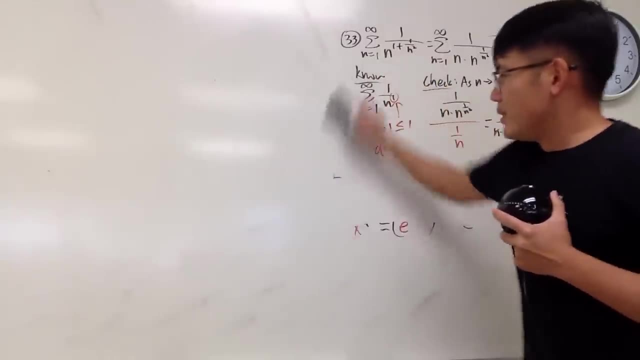 Cool. So now we did a lot of questions: How much time is this? 2 hours and 30 minutes, I feel it. I'm not going to lie. I feel like, oh, okay, It's kind of tiring. 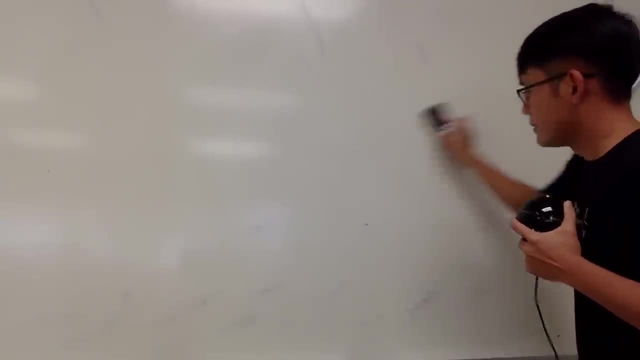 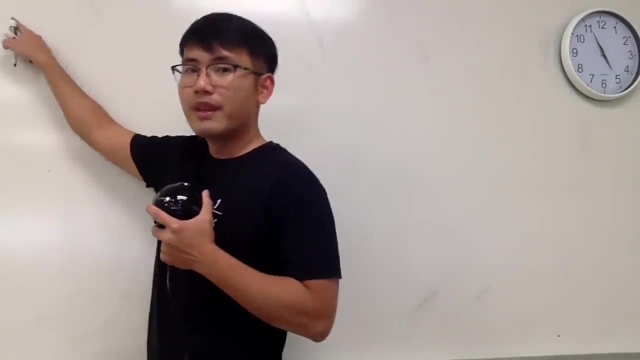 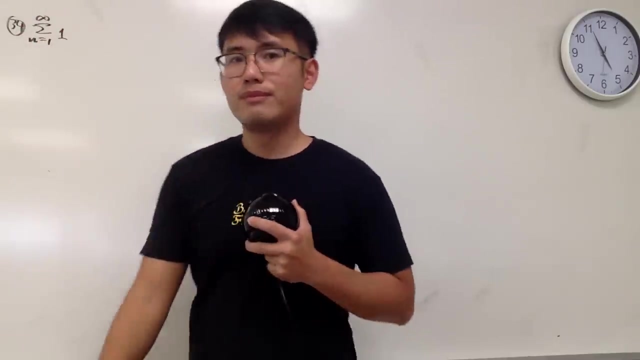 But it's okay. Okay, That was number 33.. Now let's do number 34.. Number 34, we have to do the sum as n goes from 1 to 0.. Let's do the sum as n goes from 1 to infinity of 1.. 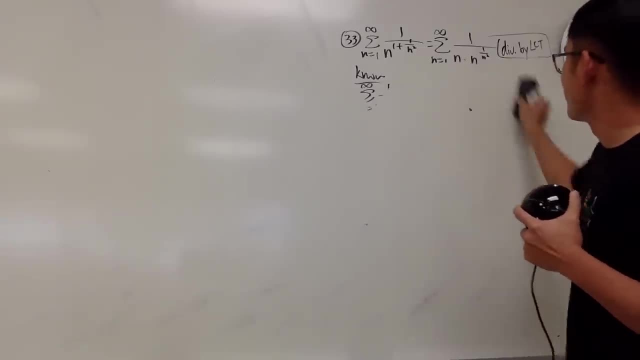 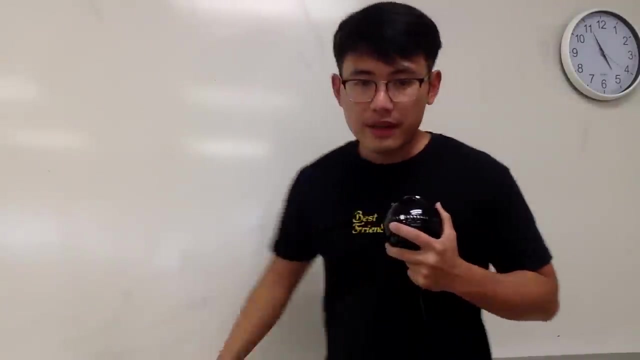 I feel it, I'm not going to lie- I feel like, oh, okay, it's kind of tiring, but it's okay. Okay, That was number 33.. Now let's do number 34.. Number 34,: 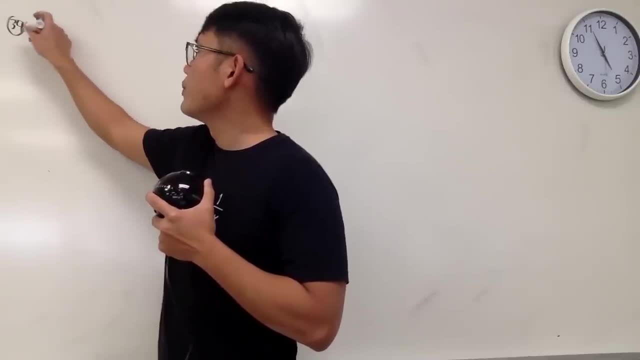 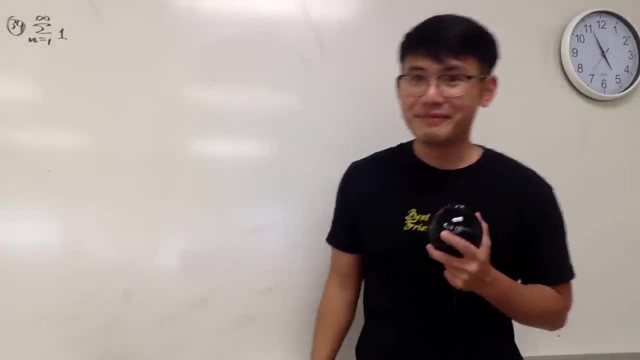 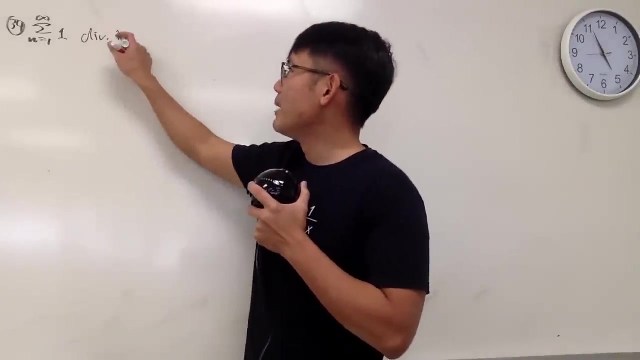 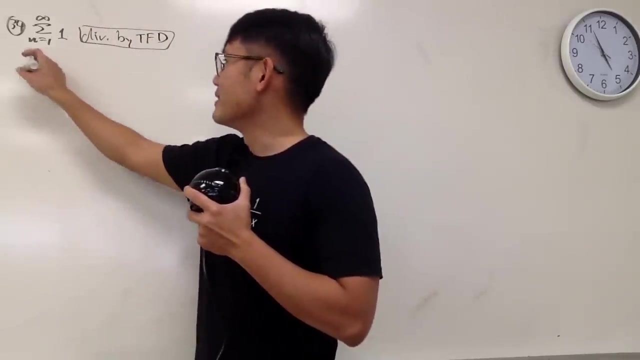 we have to do the sum as n goes from 1 to infinity of 1.. What's the answer? Diverges This right here? diverges Why? By the test for divergence in your head, Because you can see that. 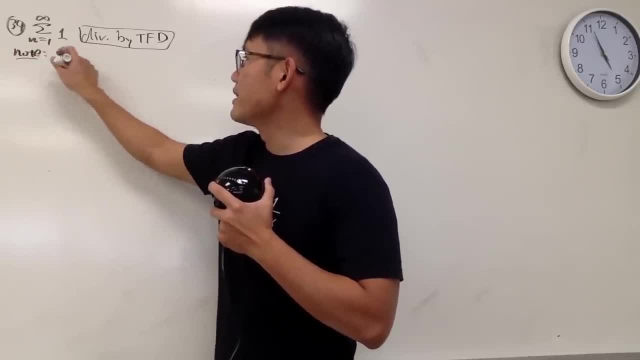 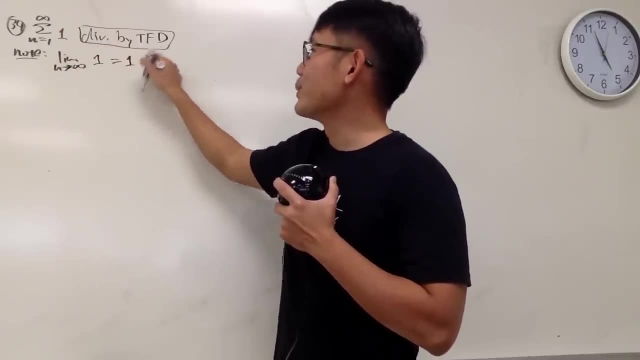 well, note, if you take the limit, as n goes to infinity, of a n which is just 1,, this is 1, and this is 9, equal to 0. So done, Okay, So that was fun. 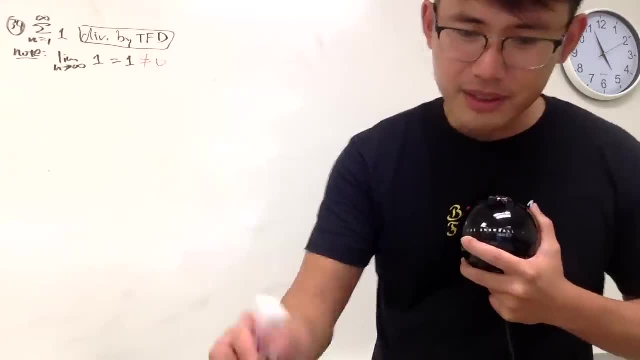 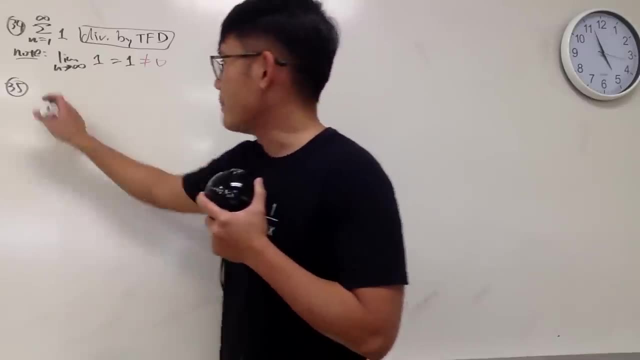 That was very, very nice. Now let's do this, number 35. This is similar to one of the questions, actually two of the questions- that we did earlier. We will have the sum as n goes from 1 to infinity. 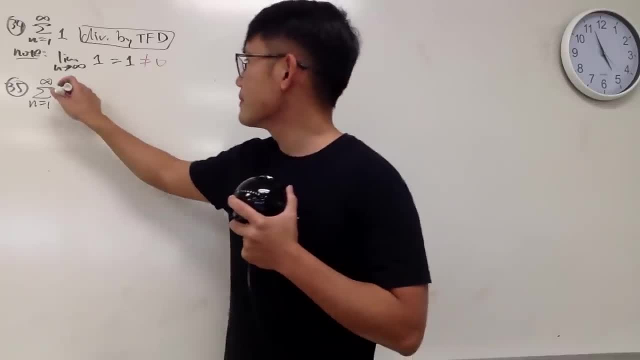 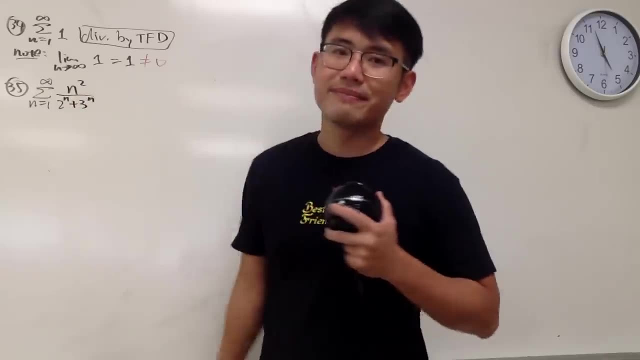 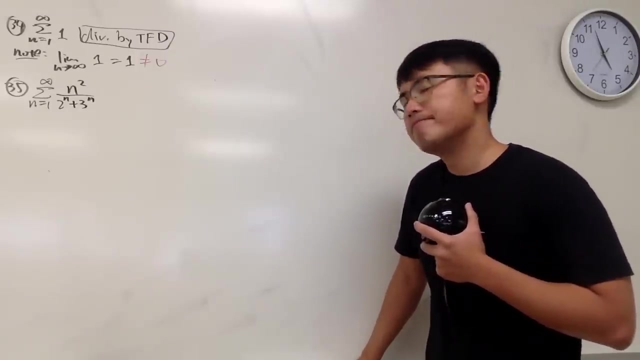 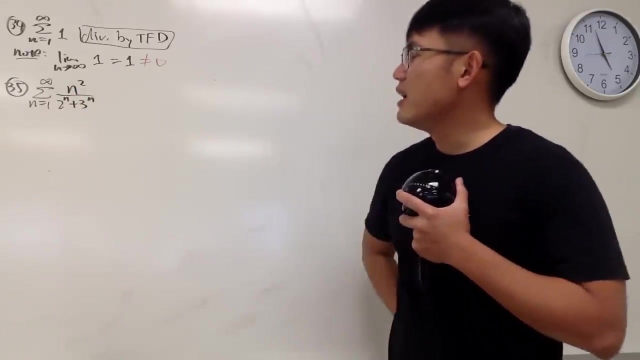 and we have n squared over and we have 2 to the n plus 3 to the n, like this: Okay, Does it converge or does it diverge? Well, on the bottom, the dominating power will be just 3 to the n. 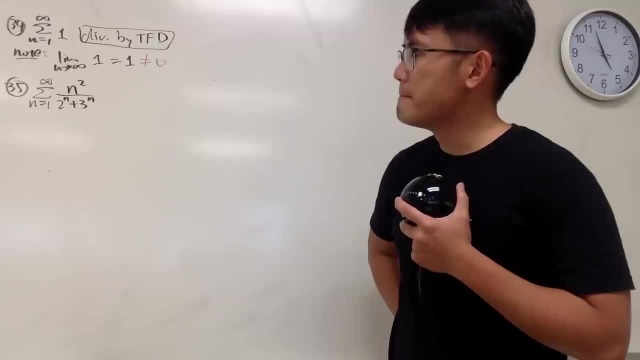 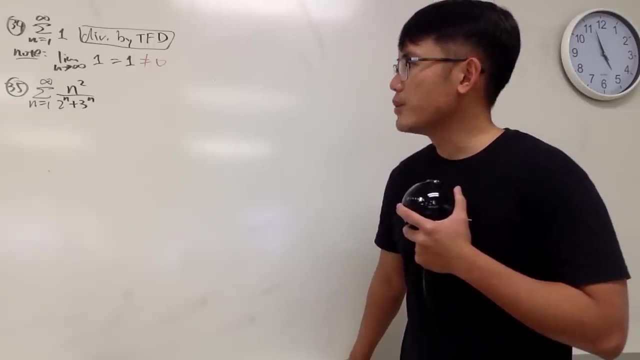 So okay, that's good news. Let's see How can we do it. Should we do the direct comparison test or should we do the limit comparison test? Well, first of all, let's make a connection, because I think 2 to the n is bothering us too much. 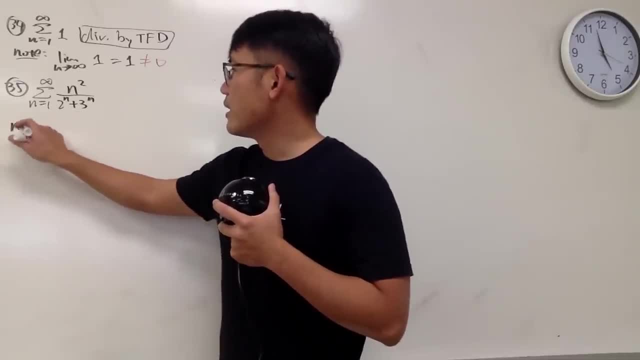 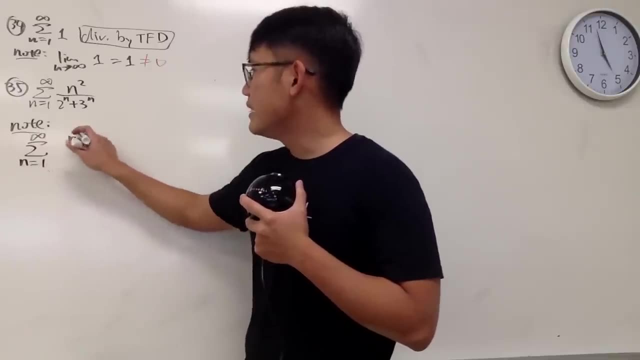 So let's see. So I'll just put down note right? So notice, if you look at the sum as n goes from 1 to infinity, n squared over, 2 to the n plus 3 to the n, just ignore the 2 to the n, right. 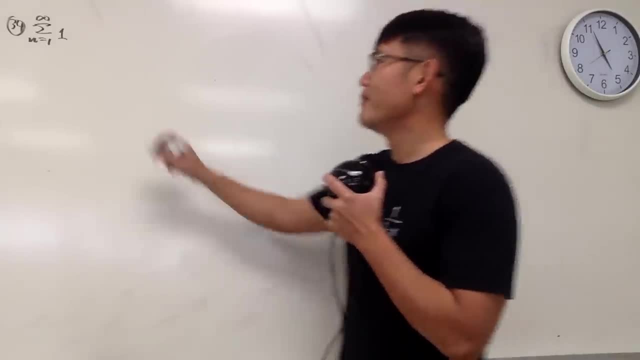 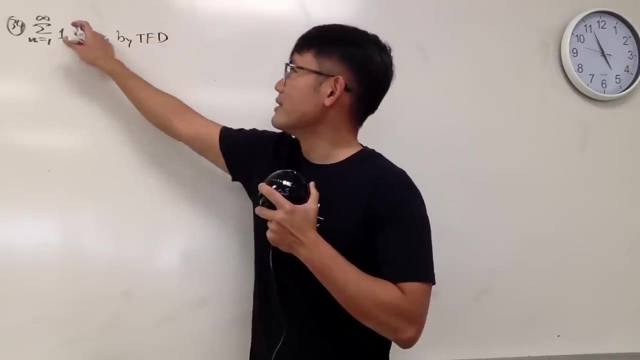 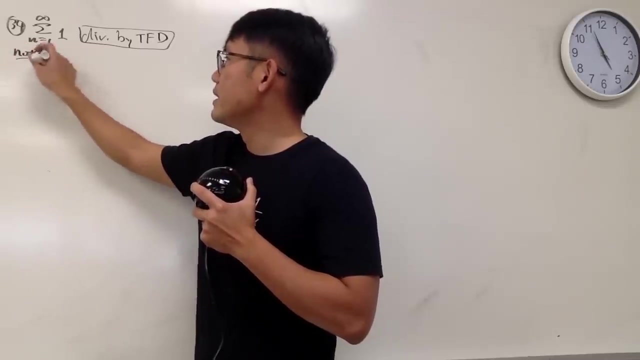 What's the answer? Diverges This right here. diverges Why? By the test for divergence in your head, Because you can see that. well note, If you take the limit as n goes to infinity, you can see that it's equal to 1.. 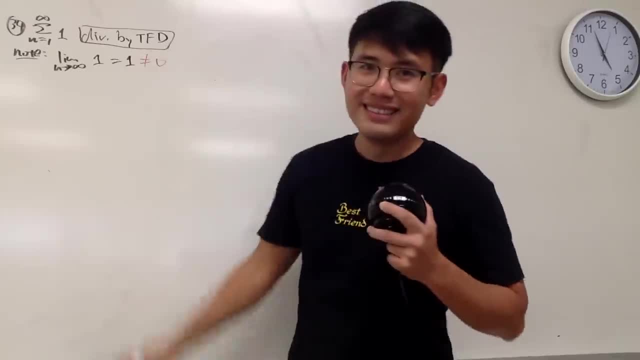 And now the answer is 1.. So we have to do the sum, as n goes from 1 to infinity, of 1.. This is 1. And this is not equal to 0. So done, Okay. So that was fun. 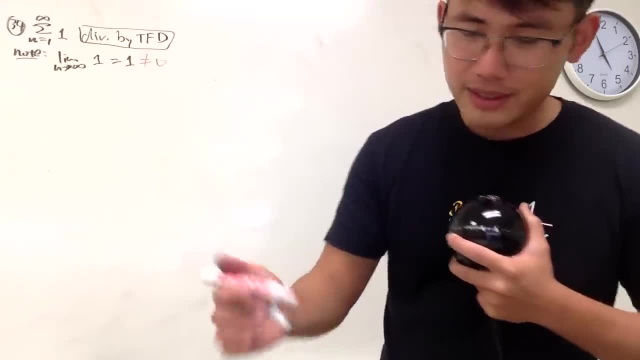 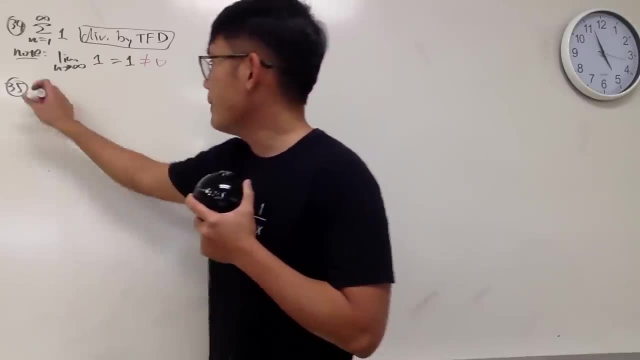 That was very, very nice. Now let's do this, Number 35.. This is similar to one of the questions, Actually two of the questions, that we did earlier. We will have the sum as n goes from 1 to infinity. 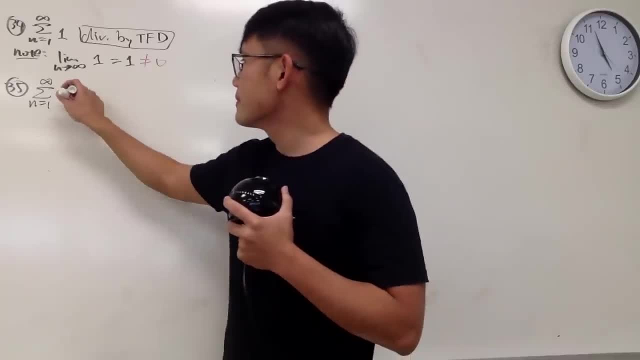 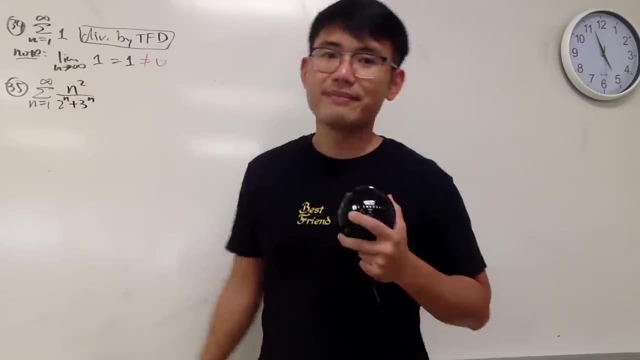 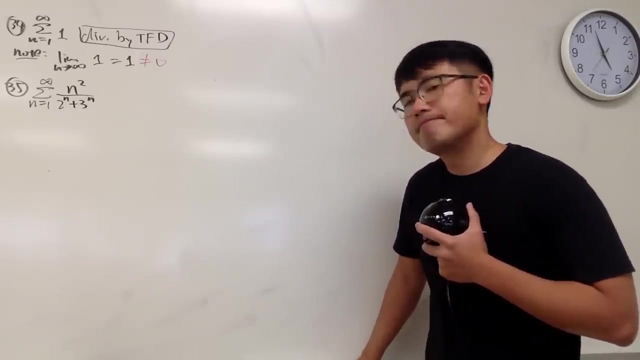 And we have n square Over, And we have 2 to the n plus 3 to the n. What's the answer? this okay, hmm. does it converge or does it diverge? well, on the bottom, the dominating power will be just 3 to the. 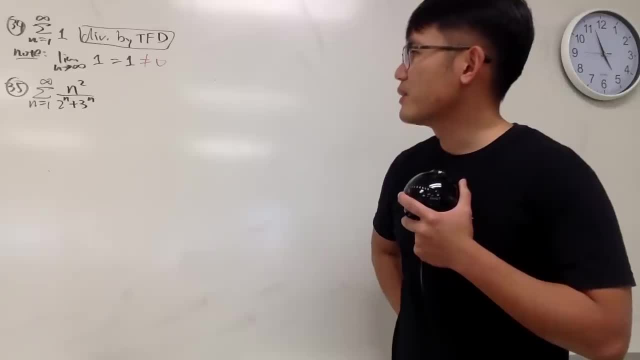 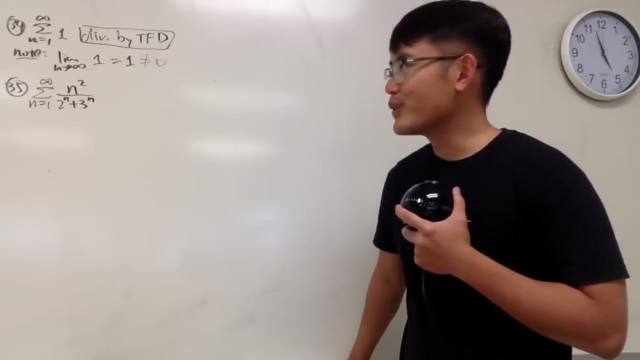 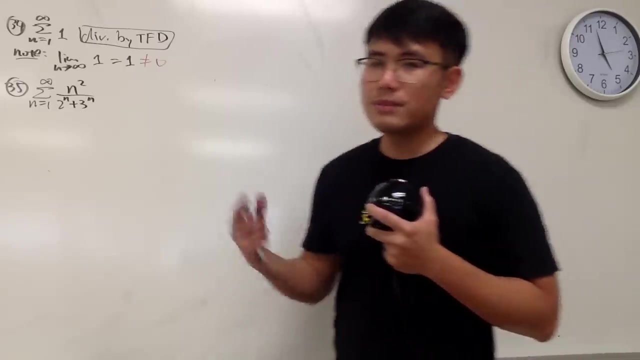 and so okay, that's good news. hmm, let's see how can we do it. shall we do the direct comparison test or shall we do the limit comparison test? well, first of all, let's make a connection, because I think 2 to the n is bothering us too much. so 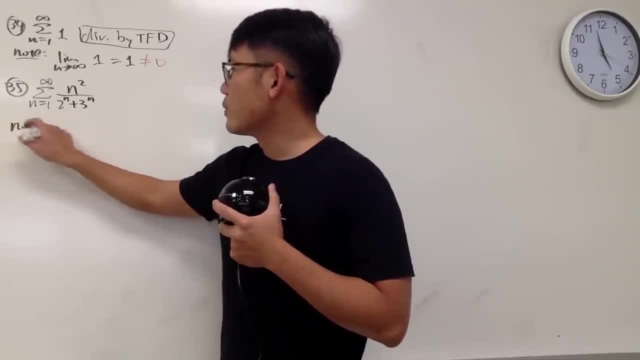 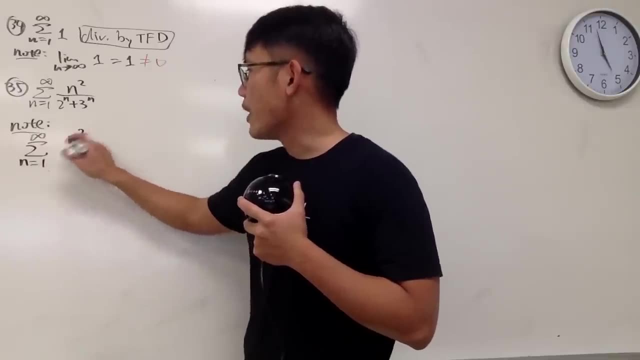 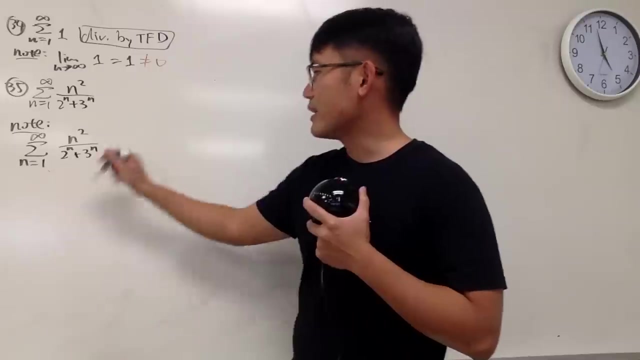 let's see, so I'll just put down note right. so notice, if you look at the sum as n goes from 1 to infinity, n squared over, 2 to the n plus 3 to the n, just ignore the 2 to the n. right, this is positive, so ignore that. 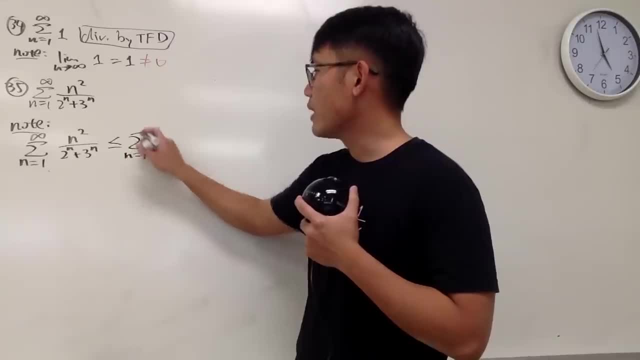 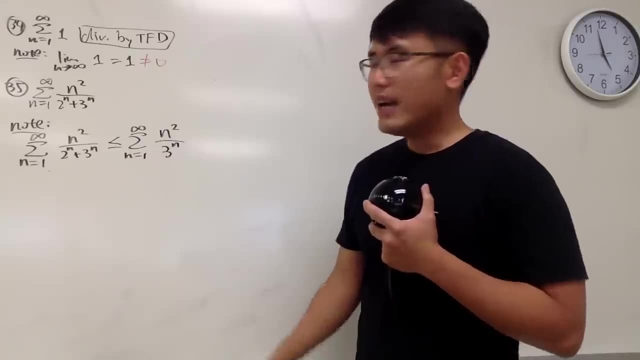 this is going to be less than or equal to the sum as n goes from 1 to infinity, n squared over 3 to the n, like this. I think this right here is slightly easier to handle and if you look back to question number 30, very similar right. you have a power. 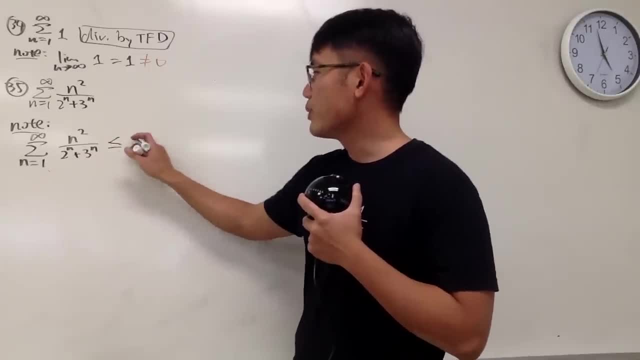 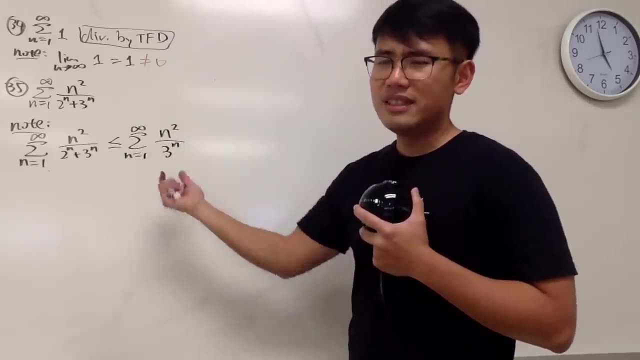 This is positive, so ignore that. This is going to be less than or equal to the sum, as n goes from 1 to infinity, n squared over 3 to the n, like this. I think this right here is slightly easier to handle. 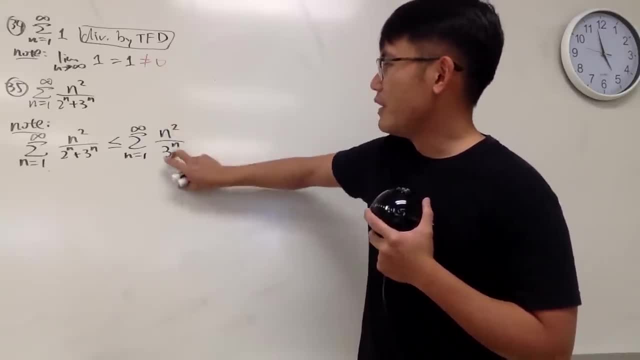 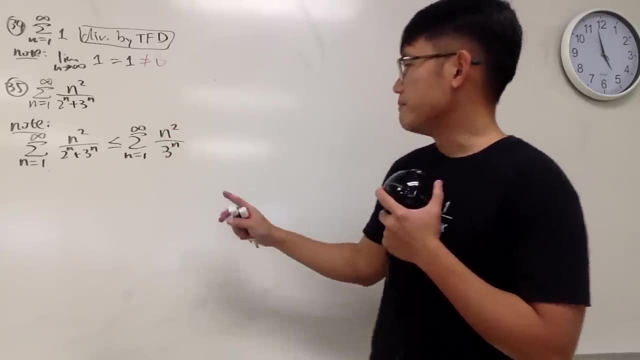 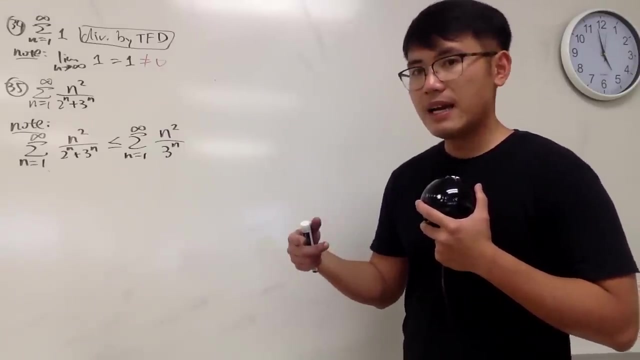 And if you look back to question number 30, very similar right, You have n to some power over 3 to some power. That was divergent. Hmm, Well, to do this, what I will show you is: let's just do the. 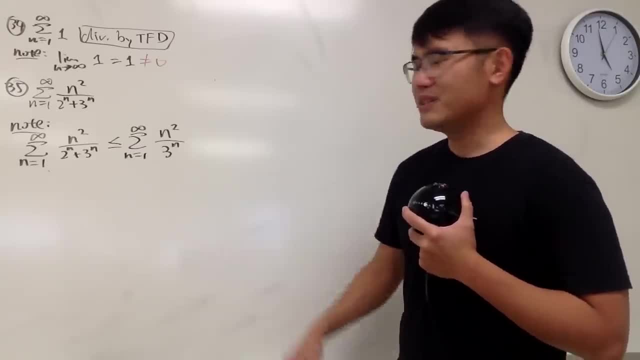 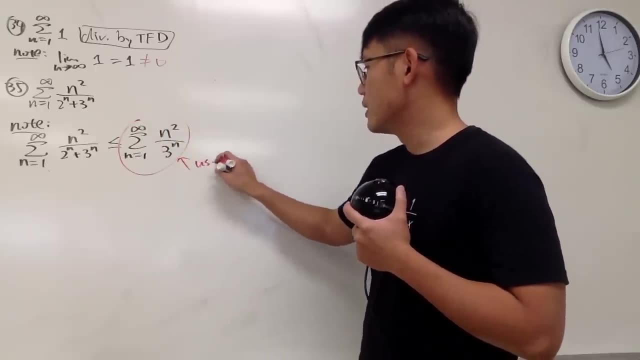 ratio test. Why not? Yeah, let's do the ratio test. So I will do the ratio test on this, right? I'll just say use ratio test Again. it's kind of weird that I didn't use the ratio test right in the beginning. 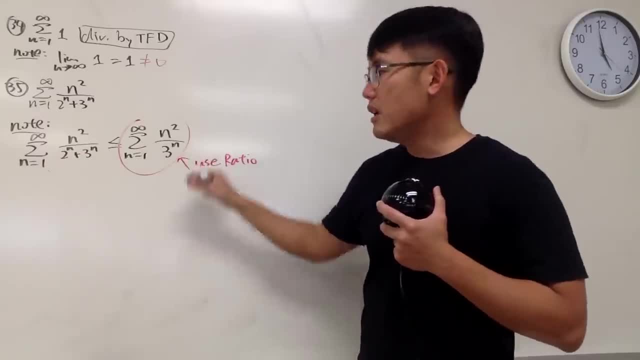 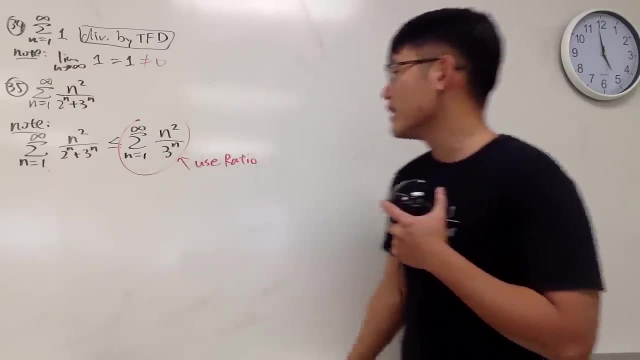 It's because I just want to simplify this a little bit. Hopefully this right here converges. If so, we can also argue that this converges because this is less than that right. So we use ratio test for this. Let's see. 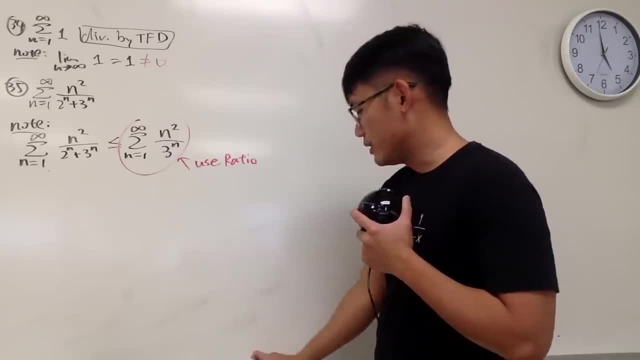 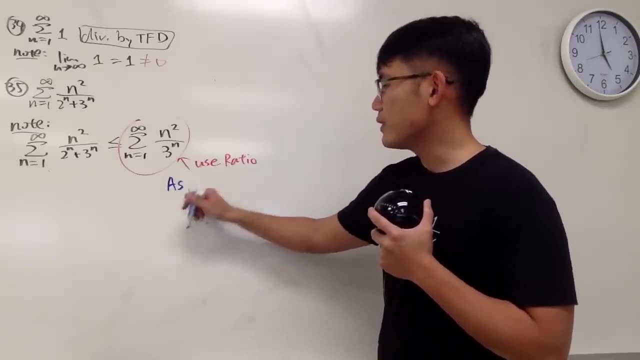 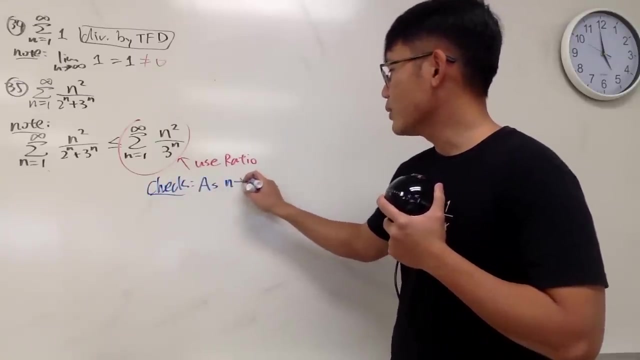 Hmm, Let's see, I will just do this in blue. I guess I will go ahead and say as n goes to. Oh, I forgot to write down the word check. We check as n goes to infinity, And now we are going to just look at this. 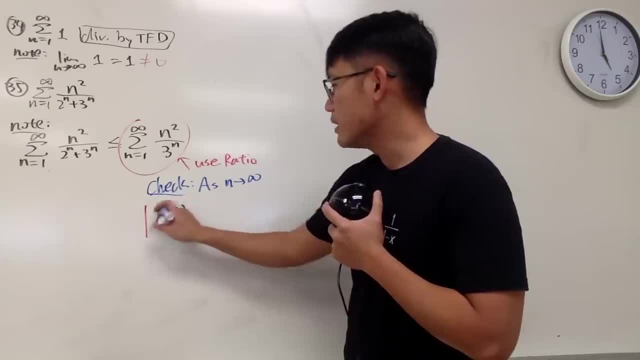 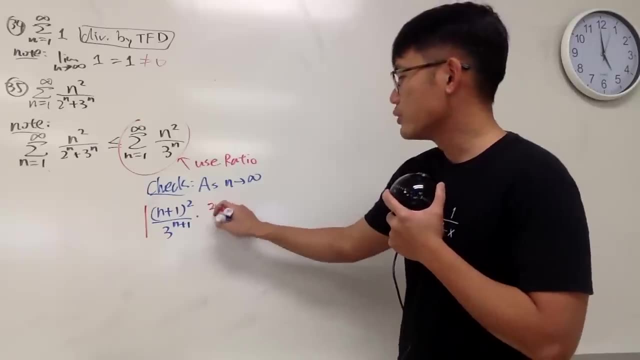 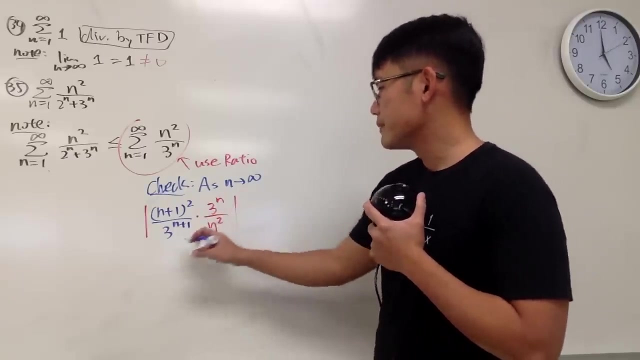 Take the absolute value n plus 1 squared over 3 to the n plus 1 times the reciprocal of the original, which is 3 to the n over n squared Like that, right? Okay, so this is nice. This is just 3 to the n times 3.. 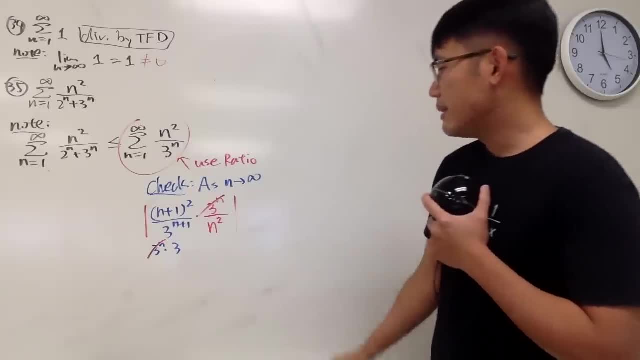 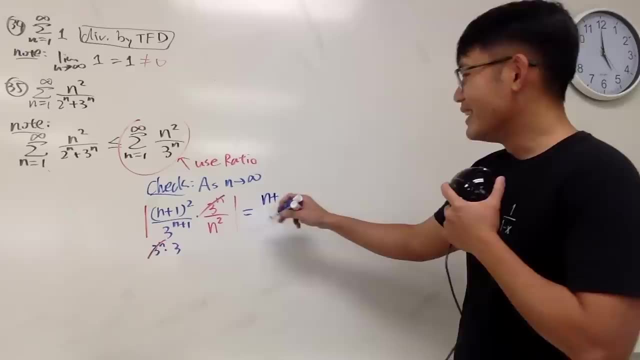 So this and that cancel. That's nice, And perhaps I'll write this down right here for you guys. This is equal to. Everything is positive. It doesn't matter what the negative Of the negative Of the absolute value. We have n plus 1 squared over 3n squared. 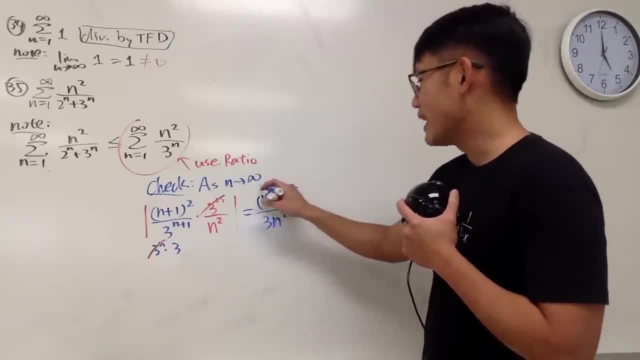 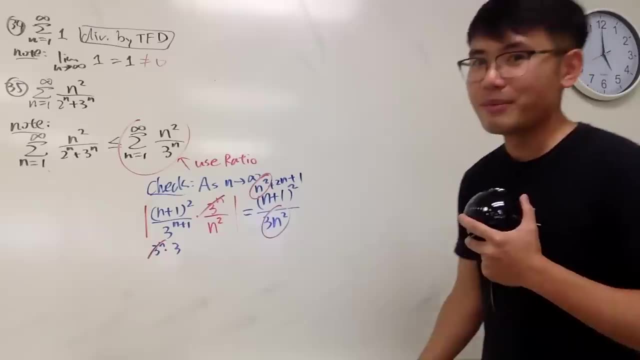 Like that. And the deal is that on the top we can multiply this out, which is n squared plus 2n plus 1.. And you see this and that are dominating parts. So we can argue that this right here. 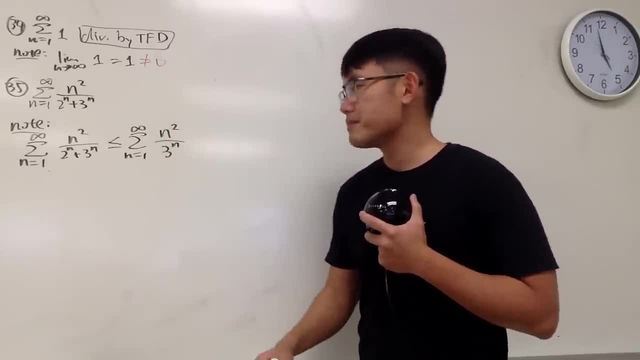 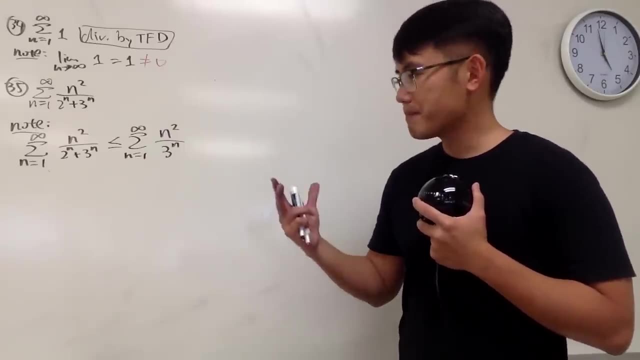 n to the sum power, over 3 to the sum power. that was a divergent. hmm well, this is F lazy. so yeah, this iski. so this is a two throw. but what this is what this is getting as well, and we're stuck at a point where it becomes a equation. because why the 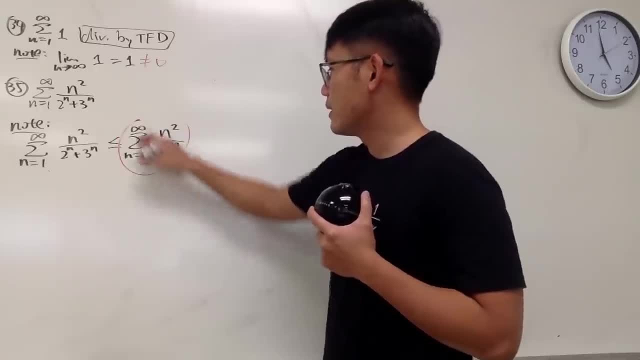 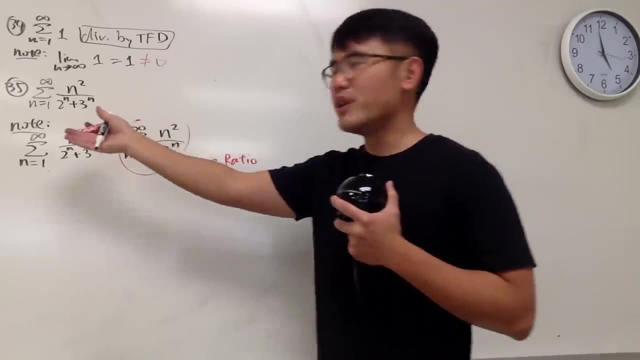 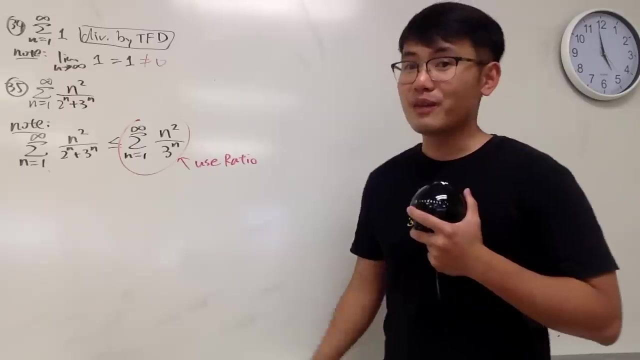 rule- let's not go back and drying all the totalרת the spin equally equal to denotation brighten initial is equal to 2. so in fact, to do this while will show you is: let's just do the visual test, point, not yeah, let's do a real test. so I would do the visual test on this, like want to say use ratio Tests again, it's kind of work either you use a real test Right in the beginning. it's because i just want to simplify this a little bit. over the shruged yes, if so, we can also get a jerk rank against this. but I hope this right here converges. if so, we can also also get this right here converges. if so, we can also solve this expression here- is because the we won't have one fewer or relatively more squared subscribers, but those are part of this boundary. so 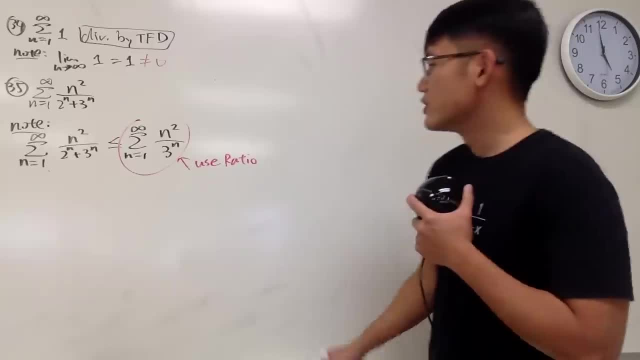 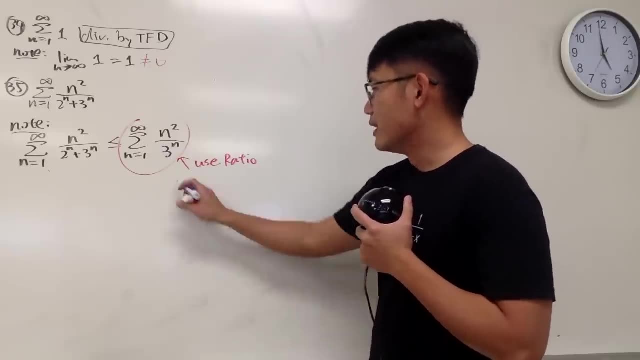 argue that this converges, because this is less than that right. So we use ratio test for this. let's see. hmm, let's see. I will just do this in blue. I guess I will go ahead and say: 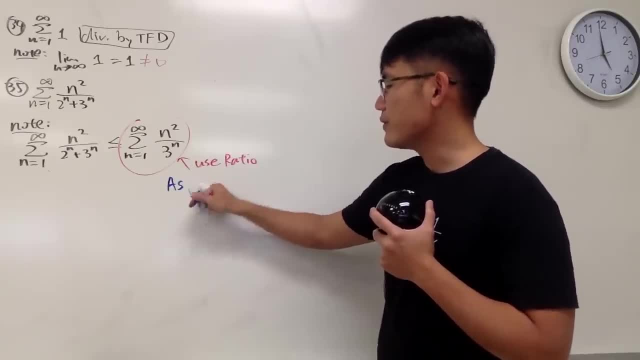 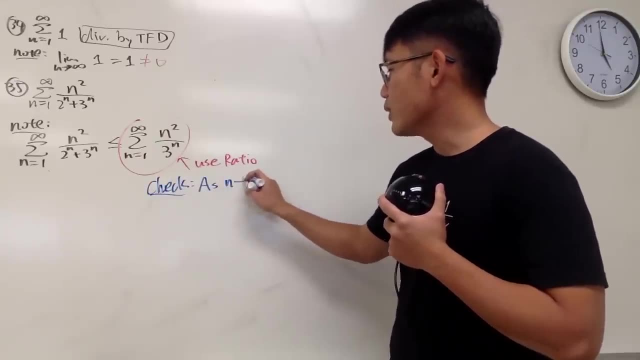 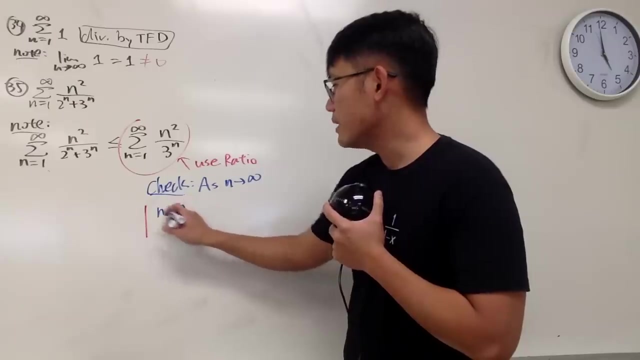 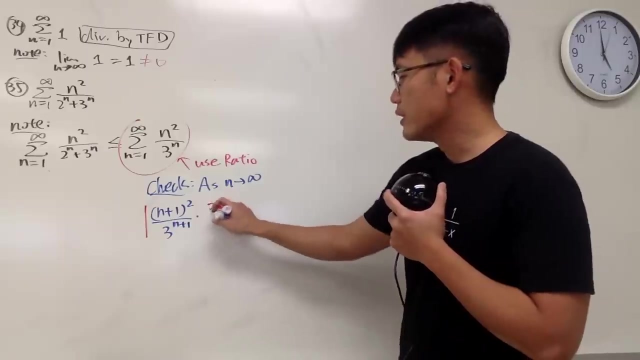 as n goes to. oh, I forgot to write down the word check. we check as n goes to infinity. and now we are going to just look at this. take the absolute value n plus 1 square over 3 to the n plus 1 times the reciprocal of the original, which is 3 to the n. 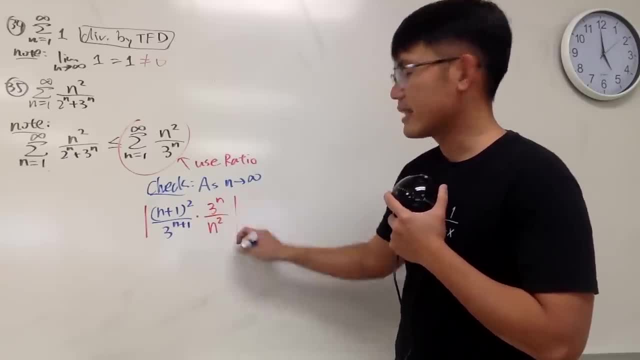 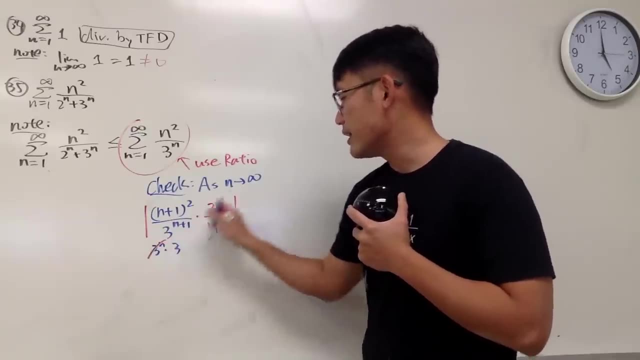 over n square like that, right? Okay, so this is nice. this is just 3 to the n times 3, so this and that cancel. that's nice, and perhaps I'll write this down right here for you guys. 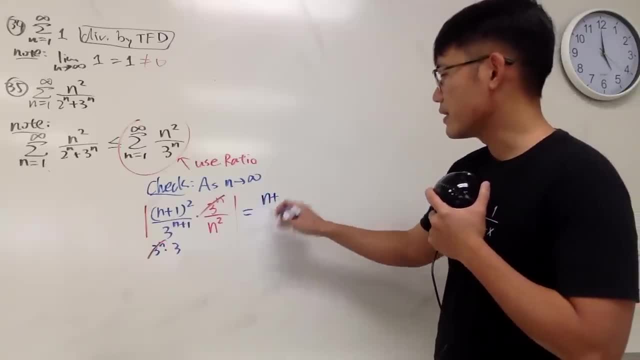 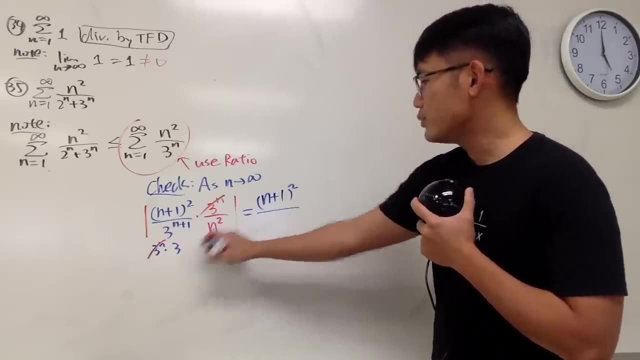 this is equal to. everything is positive, doesn't matter of the negative, of the absolute value. we have n plus 1 square over 3 to the n plus 1 times the reciprocal of the original. we have n plus 1 square over 3, n square like that, and the deal is that on the top, 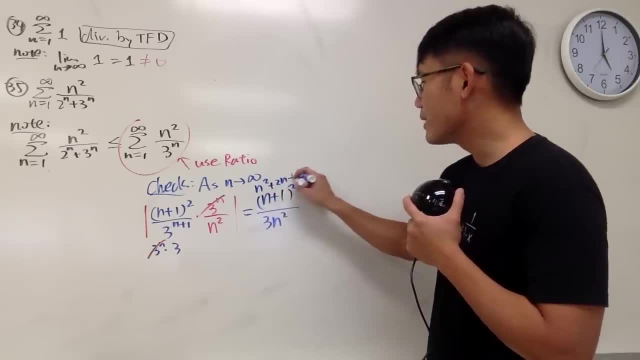 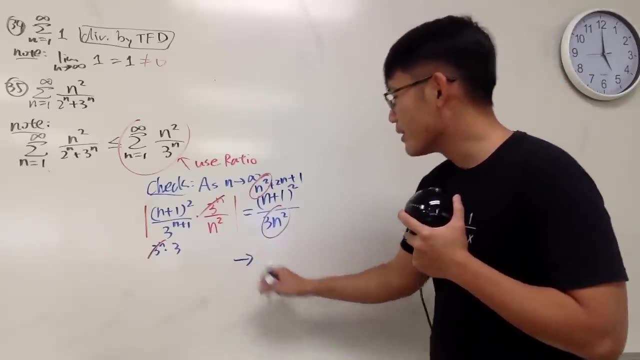 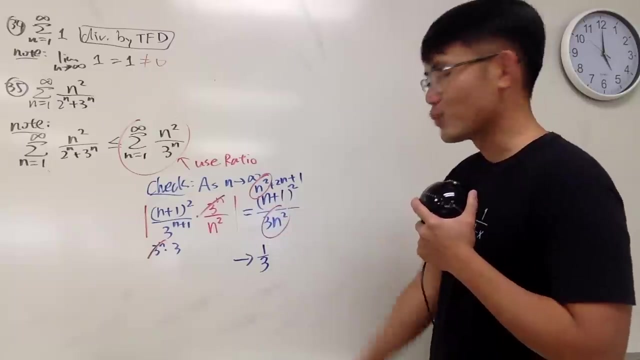 we can multiply this out, which is n square plus 2, n plus 1, and you see this, and that are dominating parts. so we can argue that this right here, this right here, approaches 1 third. right, because they have the same power, it's just 1 third, and the good thing is that this 1 third 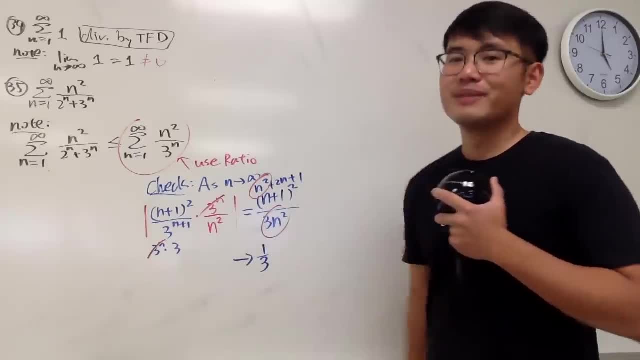 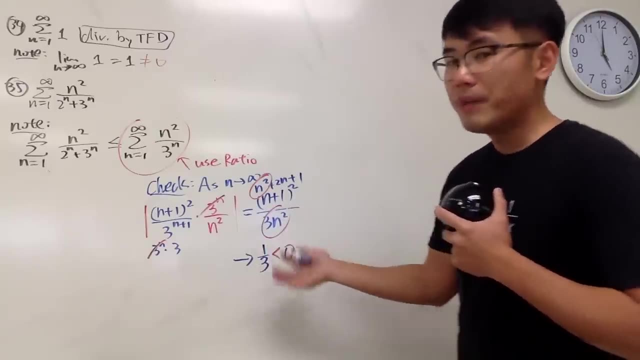 This right here approaches 1 third. Right, Because they have the same power. It's just 1 third And the good thing is that this 1 third is less than 0. So, based on the ratio test, we know this right here converges: 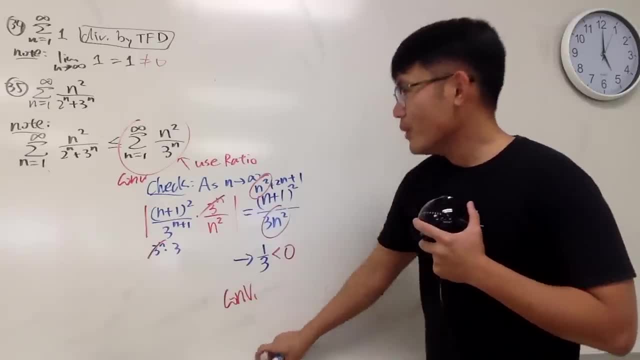 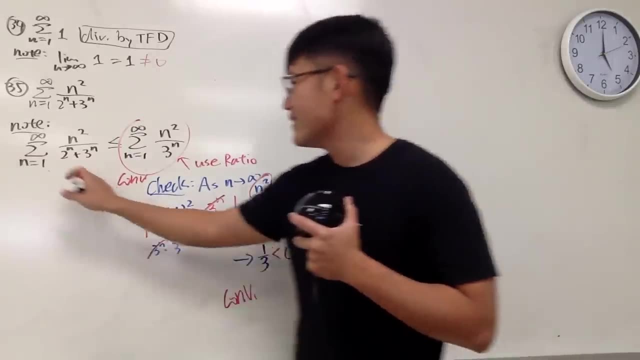 Right. So this right here converges. So now, once you prove that this right here converges, we can come back here and say this: right here also converges. Right, Because we have this inequality that we set up. I'll just put down: also converges. 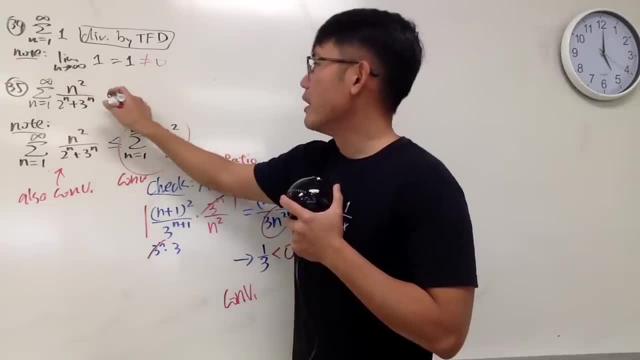 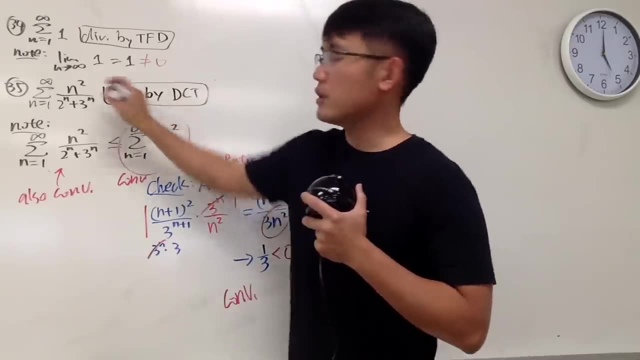 And of course, I will come back here and say this right here: converges by the direct compression test. What's this? What's this And how do we know this? converges Because we used the ratio test, So we used both in this question, right here. 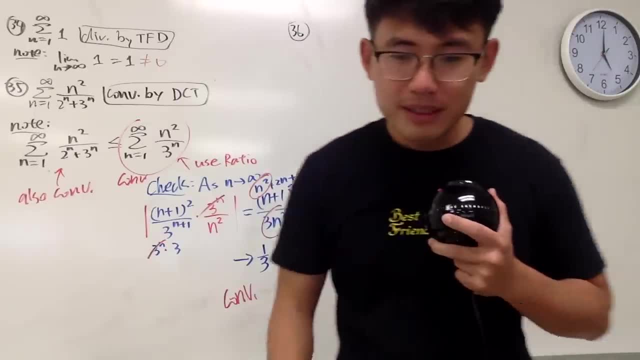 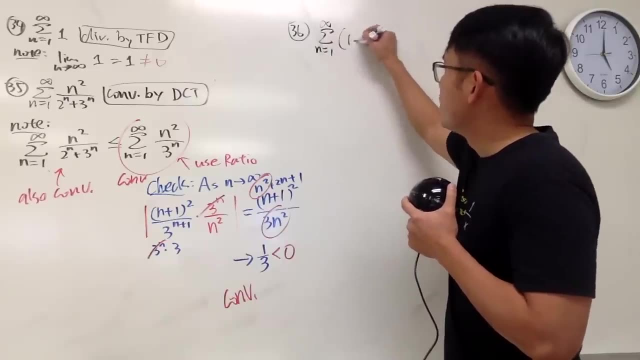 So that's very nice, Right? So here we go, Number 36.. All right, The sum as n goes from 1 to infinity of 1 minus 1 over n to the nth power, like that. Hey, hey, hey, hey, hey. 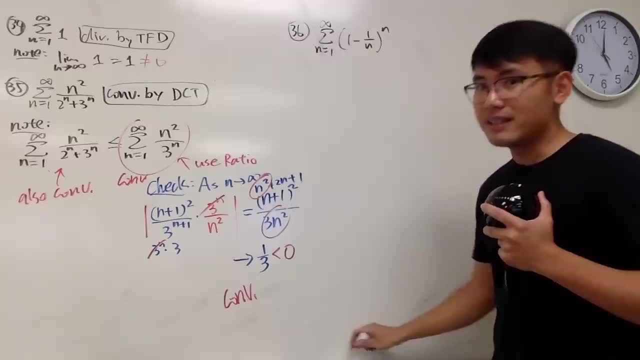 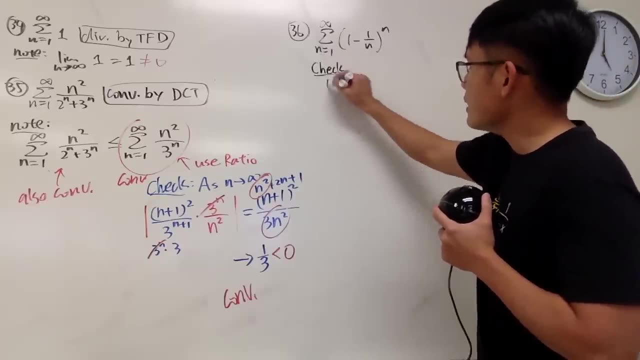 Doesn't this look like the fact? Well, the fact is about limit, So we better talk about the test for divergence first. So let's go ahead and check the limit, as n goes to infinity, of just this, which is 1 minus 1 over n, to the nth power. 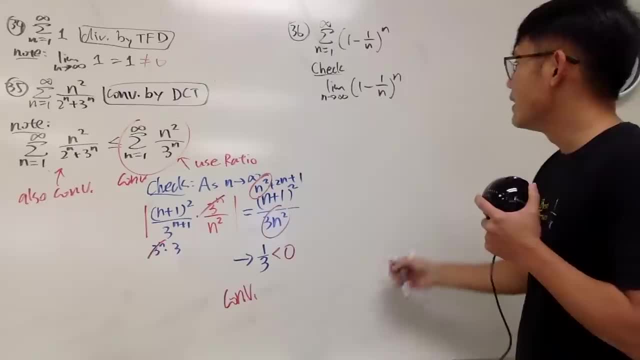 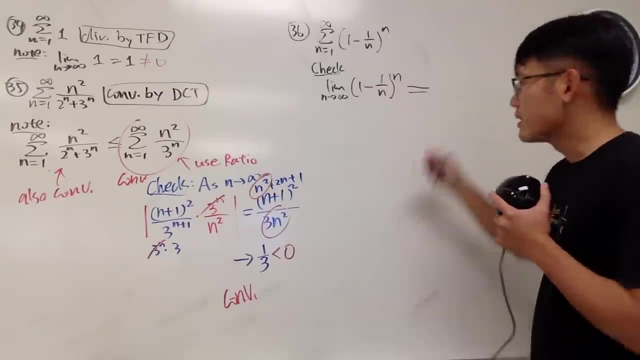 This is just the test for divergence check. Well, look at, a is actually negative 1 and b is positive 1.. So when you use the fact, indicate that a is equal to negative 1 and b is equal to 1.. 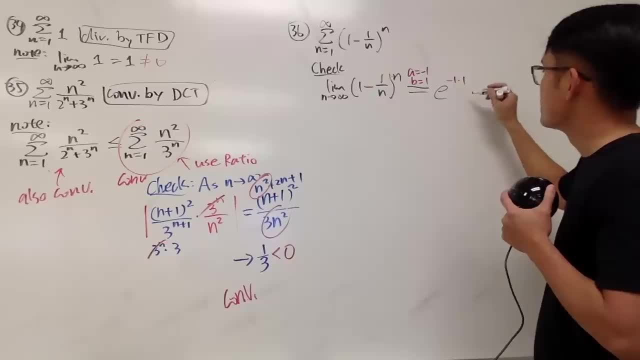 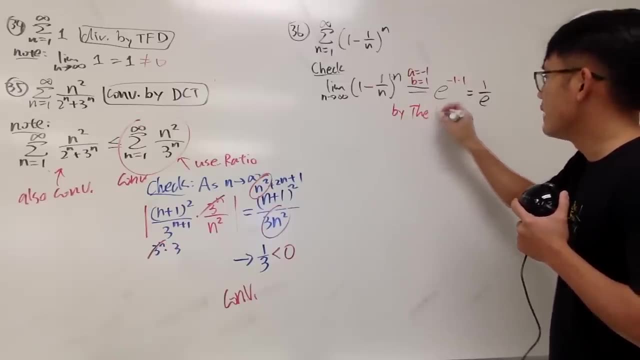 So we get e to the negative 1 times 1.. So this is just 1 over e, Right, And to do that. of course you can just call that by the fact. I don't call this the limit, because the limit is a sine theta over cosine. 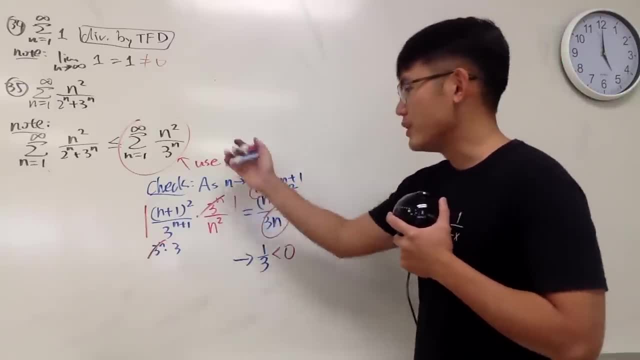 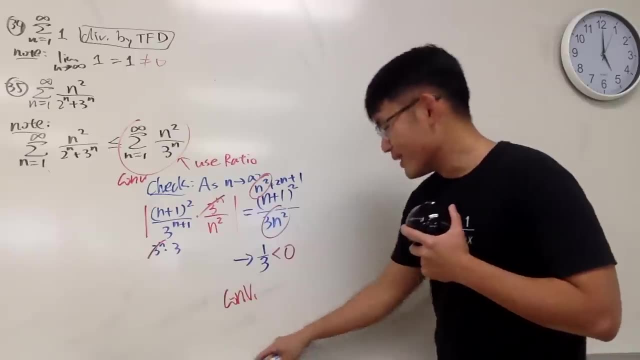 is less than 0.. So, based on the ratio test, we know this right here converges right. so this right here converges. So now, once you prove that this right here converges, we can come back here and say: 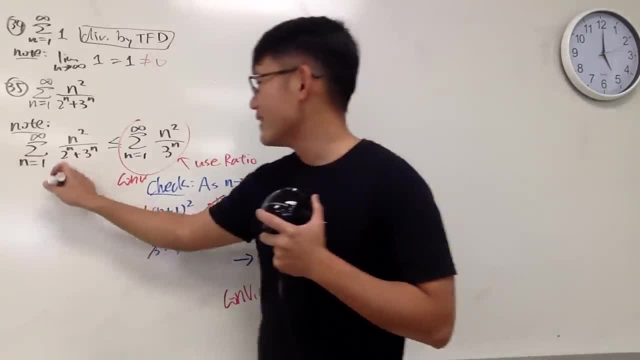 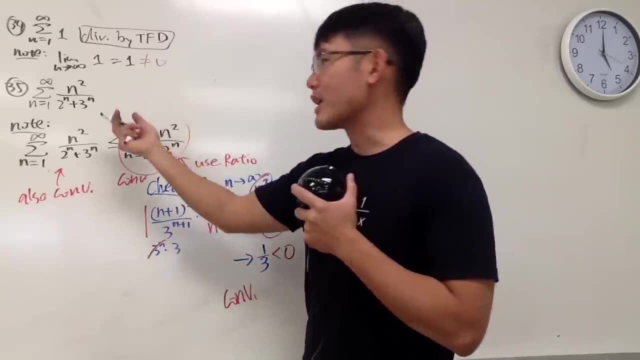 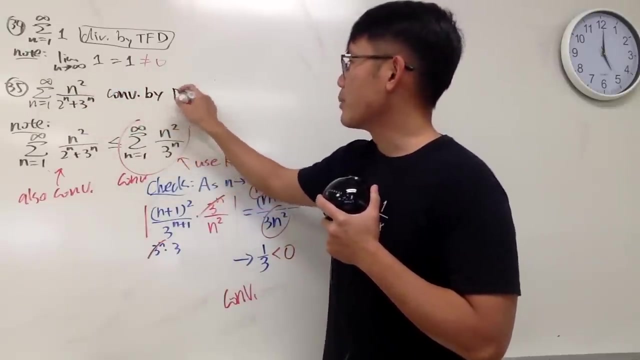 this right here also converges. right, because we have this inequality that we set up. I'll just put down: also converges and of course I will come back here and say this right here: converges by the direct compression test. what's this? what's this and how do we know this? converges. 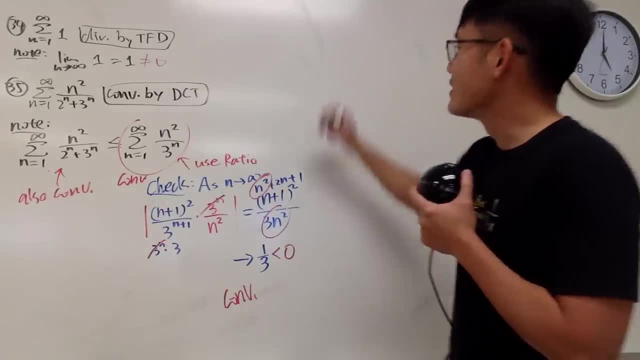 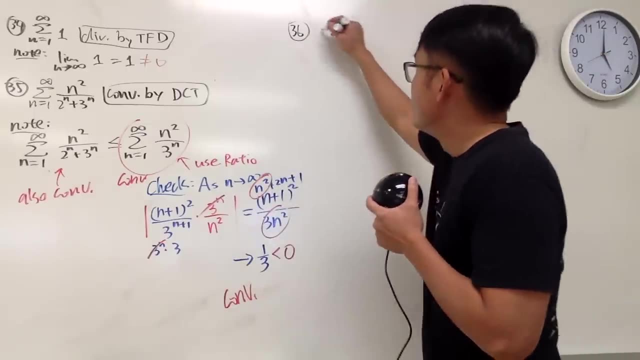 Because we used the ratio test, so we used both in this question right here. so that's very nice, right? so here we go, number 36,. all right, the sum as n goes from 1 to infinity of 1 minus 1 over n to the nth power. 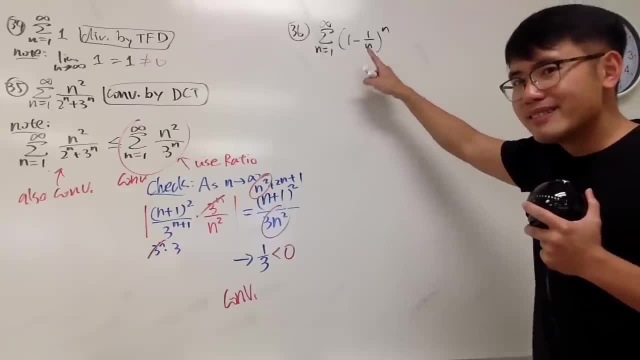 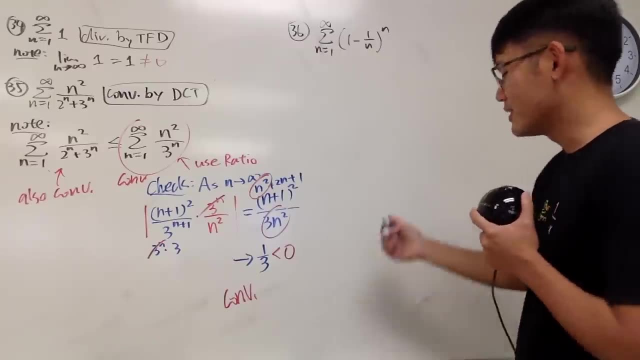 like that. hey, hey, hey, hey, hey, doesn't this look like the fact? Well, the fact is about limit, so we better talk about the test for divergence first. so let's go ahead and check the limit, as n goes to infinity of just this. 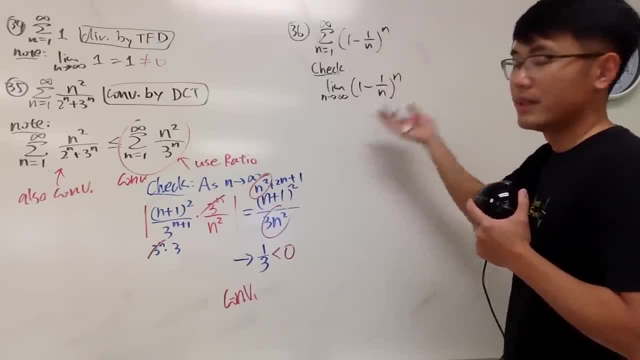 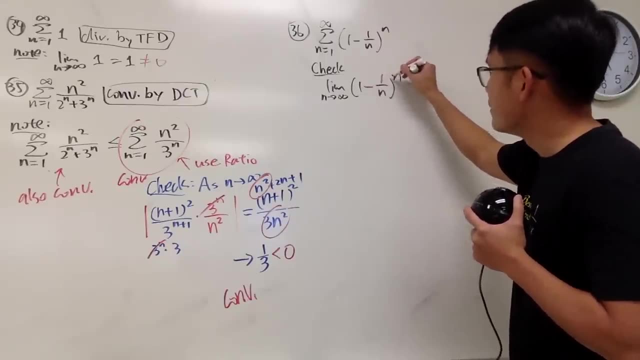 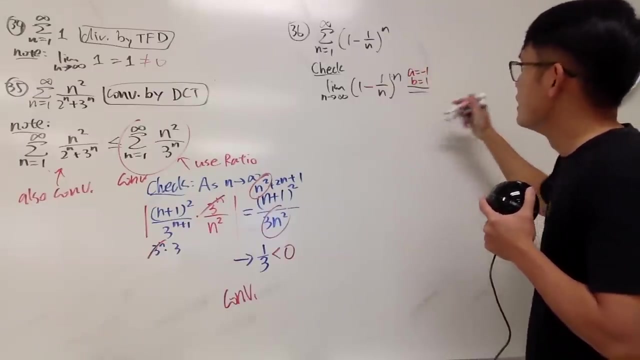 which is 1 minus 1 over n to the nth power. This is just the test for divergence check. Well, look at a is actually negative 1 and b is positive 1, so when you use the fact indicate that a is equal to negative 1 and b is equal to 1, so we get e to the negative 1 times 1,. 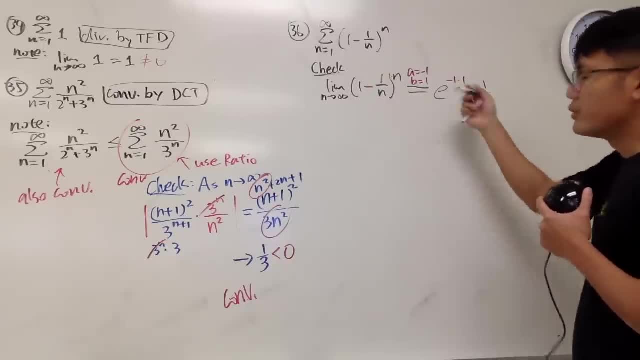 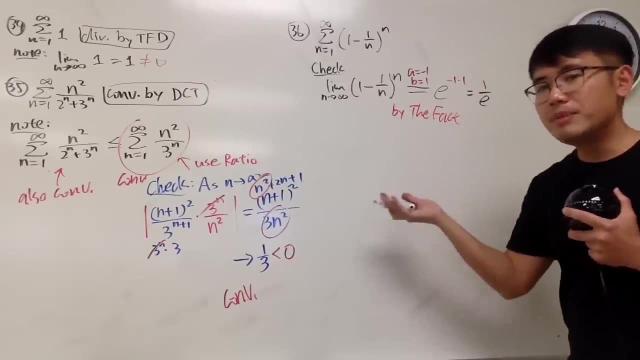 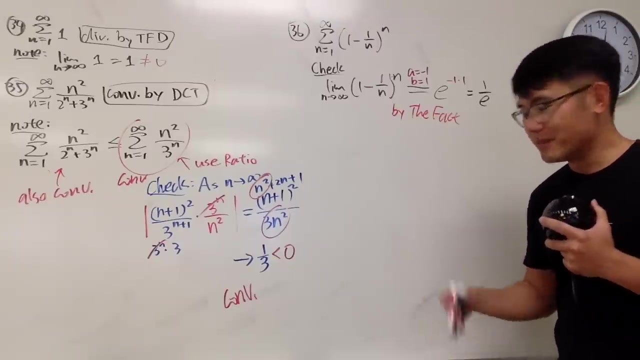 so this is just 1 over e right and to do that. of course you can just call that by the fact. I don't call this the limit, because the limit is the sine theta over cosine, sorry, the sine theta over uh, sine theta over theta, and that's like a bigger limit in my opinion. 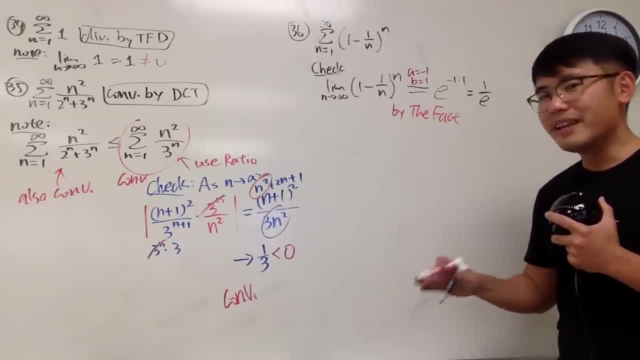 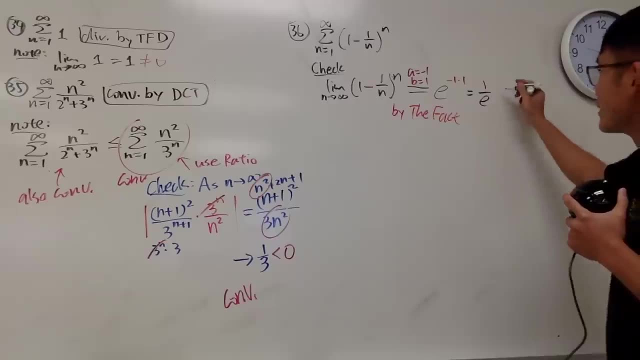 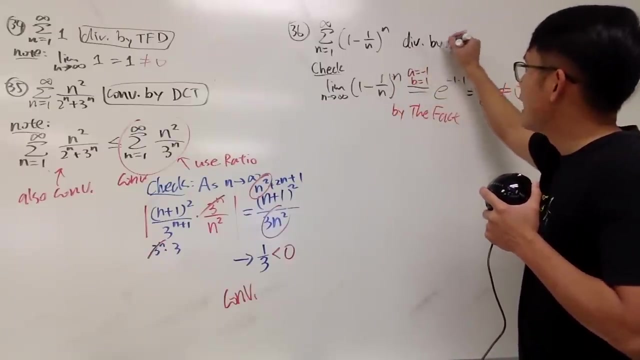 Sine theta over theta And that's like a bigger limit in my opinion. Anyway, this right here is 1 over e, But the problem is that this right here is not equal to 0. So this right here diverges by test for divergence. 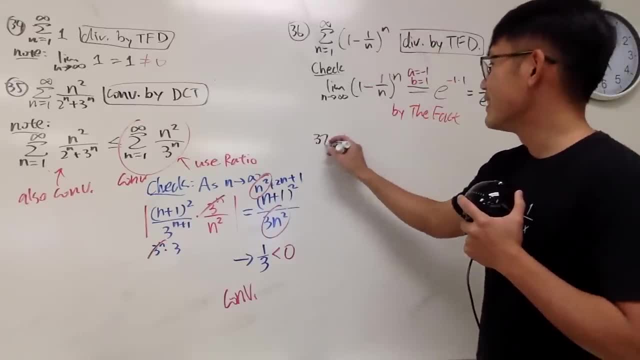 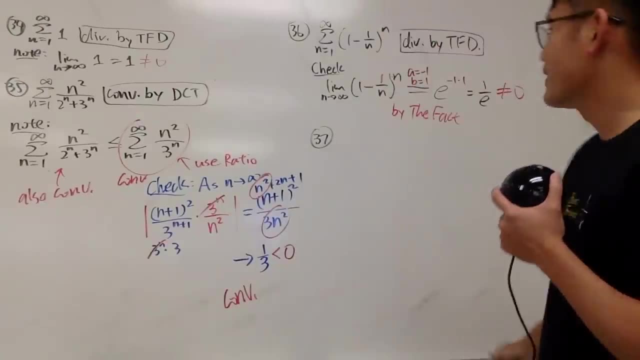 Right By test for divergence. That's it Now, number 37.. I just put that, and then we have the n squared right there, Okay, So sum as n goes from 1 to infinity: 1 minus 1 over n. 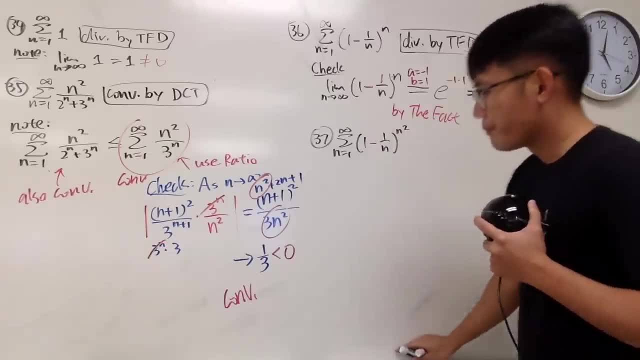 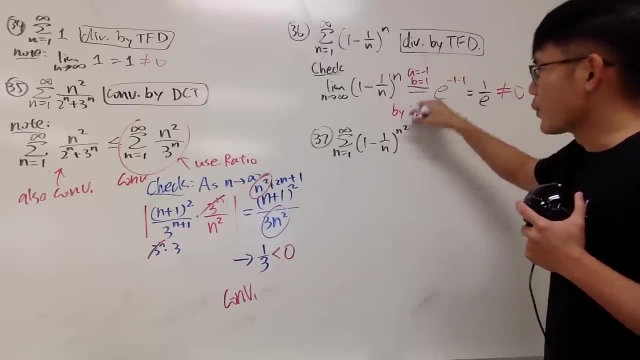 And then here we have n squared right here. Well, here's the deal. You may want to try to do this. We take the square here right. Well, if you do the square, the idea is that you have to group things. 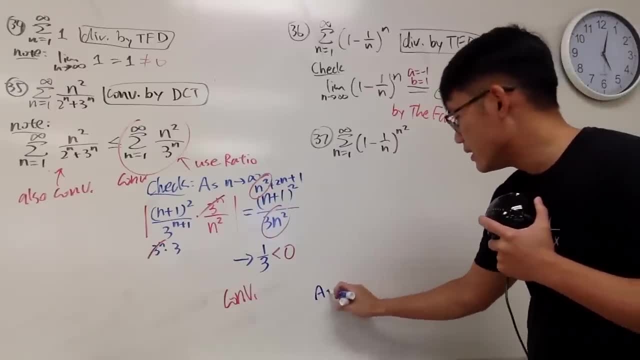 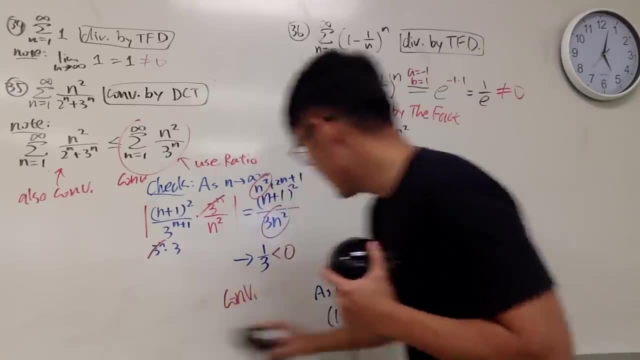 I will just put this down real quick for you, As n goes to infinity. Right, If you check this real quick, you get 1 minus. Sorry, I shouldn't, because I'm trying to do the test for divergence Limit, as n goes to infinity. 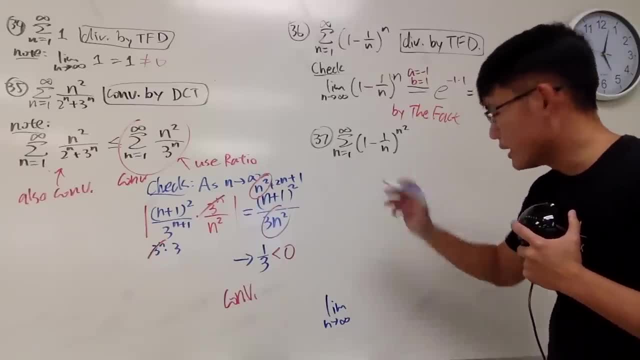 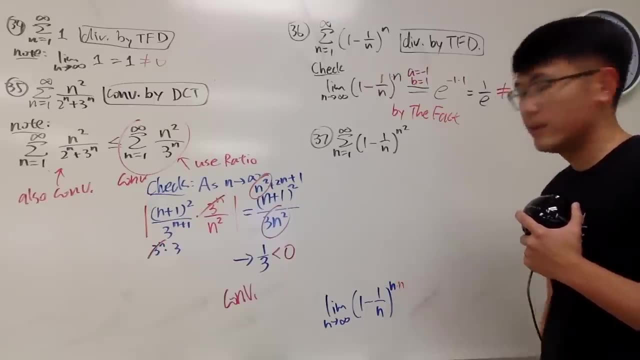 If you look at this part, if you look at this part as the following: Okay, 1 minus 1 over n n squared is the same as n times n. Right n squared is the same as n times n. For the blue part. 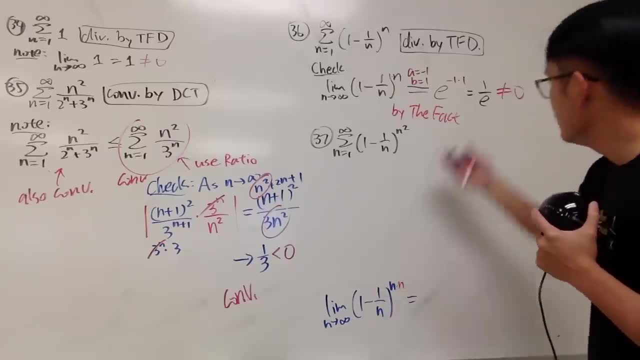 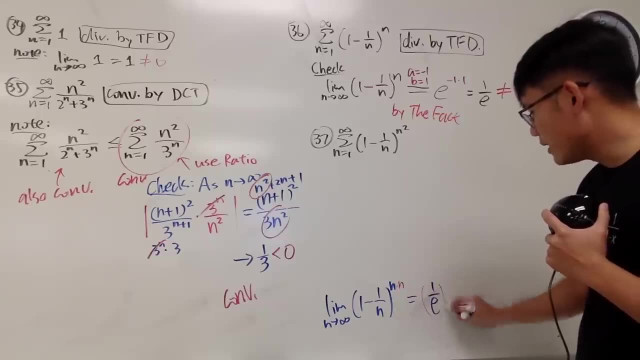 in fact you can do the following: The blue part. it actually gives you 1 over e. The blue part, And you see you still have the power n, And then, of course, you still have to do the n goes to infinity. 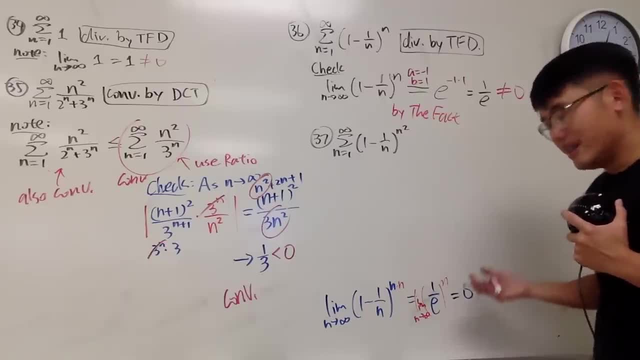 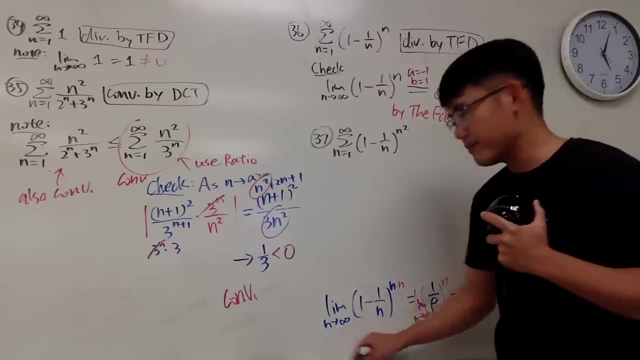 In this case, you actually end up with 0.. Unfortunately, if you do the test for divergence, in this case, 0 is a sad face. in this case, Unfortunately, What we are going to do is the root test. We want to reduce this a little bit. 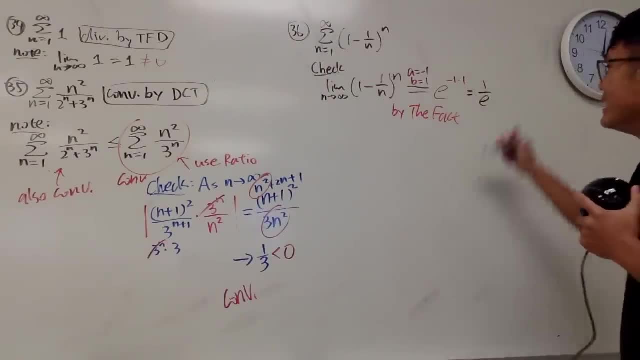 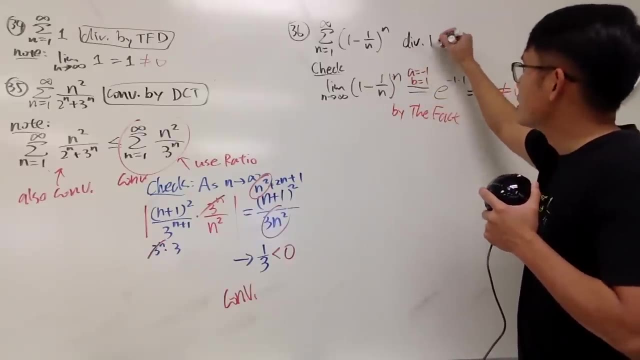 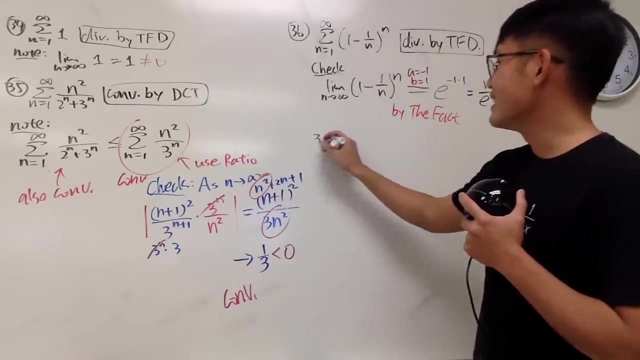 Anyway, this right here is 1 over e, but the problem is that this right here is not equal to 0, so this right here diverges by by test for divergence, right by test for divergence. that's it. 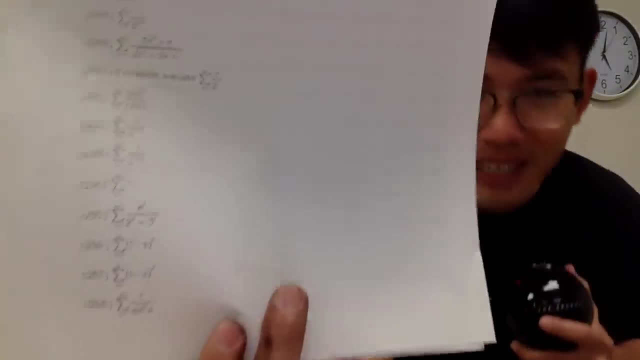 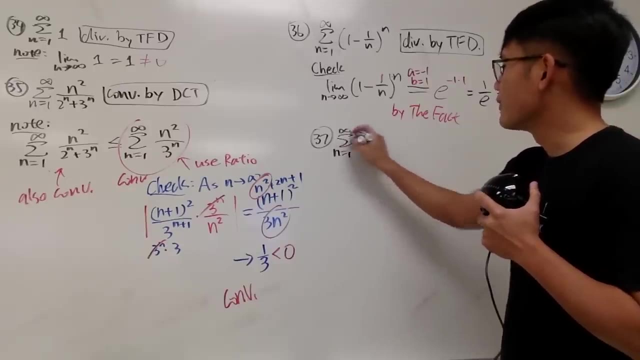 Now number 37, I'll just put that, and then we'll have the n squared right there. Okay, so sum as n goes from 1 to infinity, 1 minus 1 over n, and then here we have n squared right here. 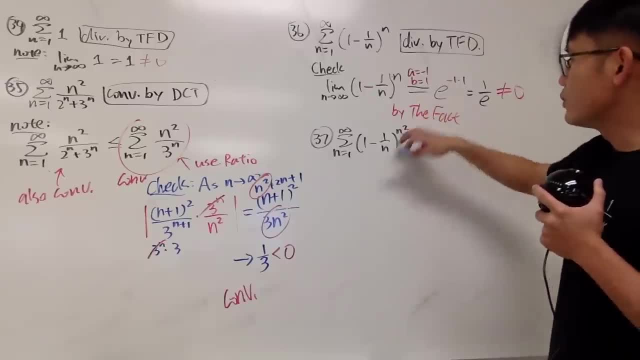 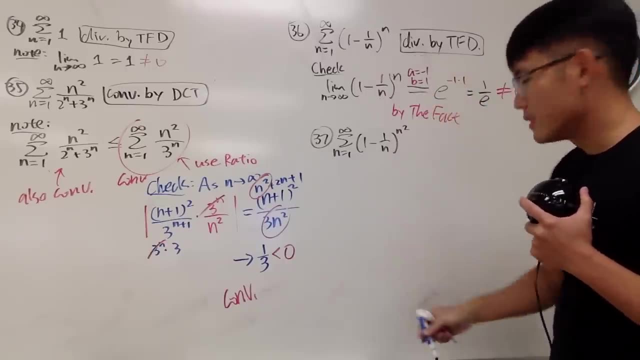 Well, here's the deal. You may want to try to do this. We take the square here right. Well, if you do the square, the idea is that you have to group things. I will just put this down real quick for you. 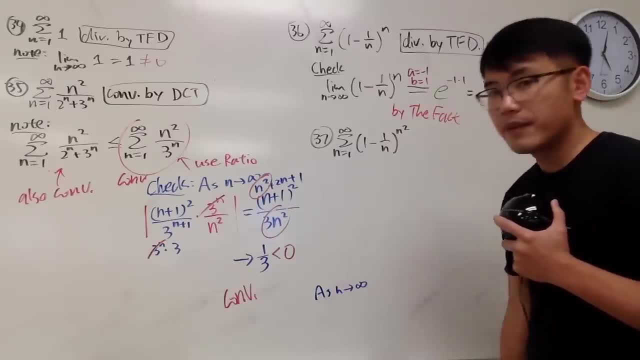 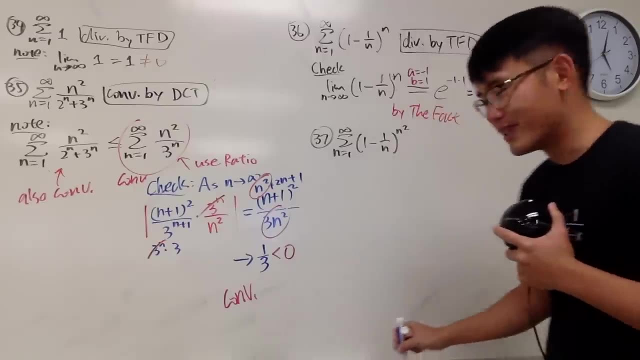 As n goes to infinity. right, if you check this real quick, you get 1 minus. sorry, I shouldn't because I'm trying to do the test for divergence Limit, as n goes to infinity if you look at this part. 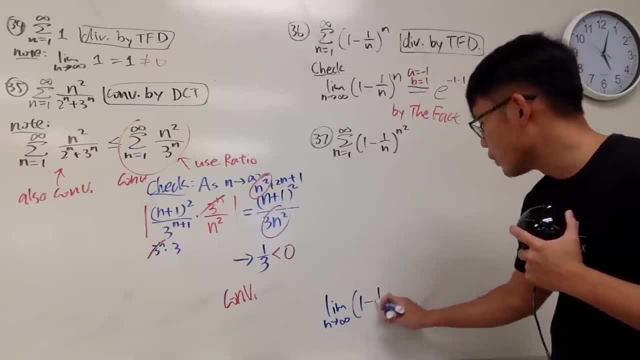 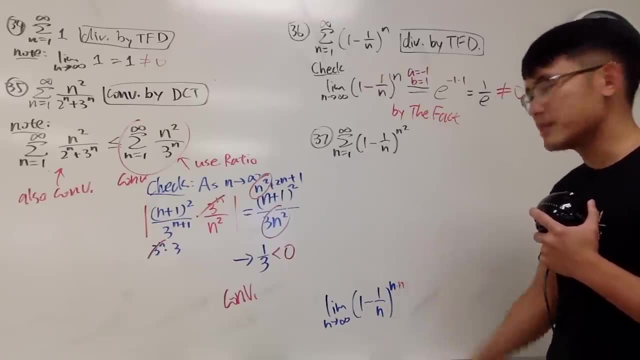 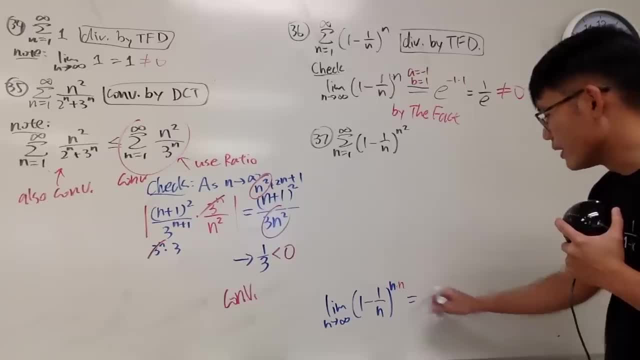 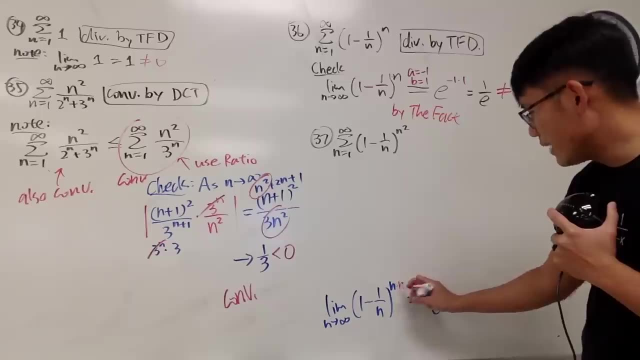 For the blue part. in fact, you can do the following: The blue part, it actually gives you 1 over e. the blue part, and you see you have still have the power n, and then of course, you still have to do the n goes to infinity. 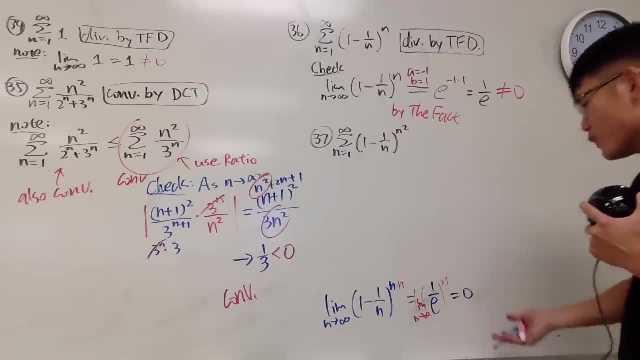 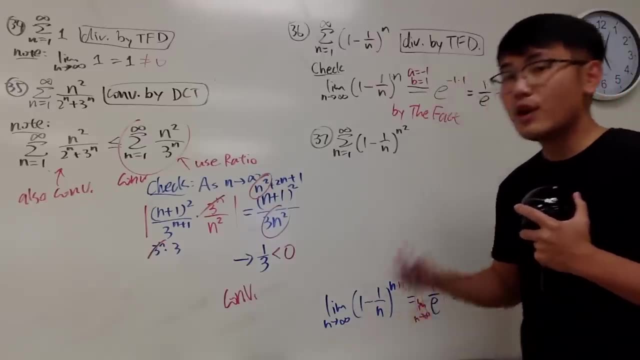 In this case, you actually end up with 0.. Unfortunately, if you do the test for divergence, in this case, 0 is a sad face. in this case, unfortunately, What we are going to do is the root test. We want to reduce this a little bit, right. 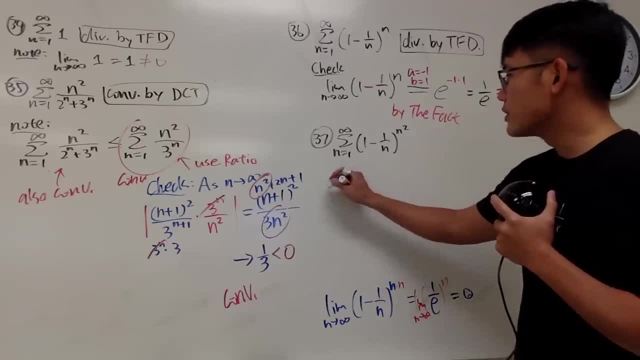 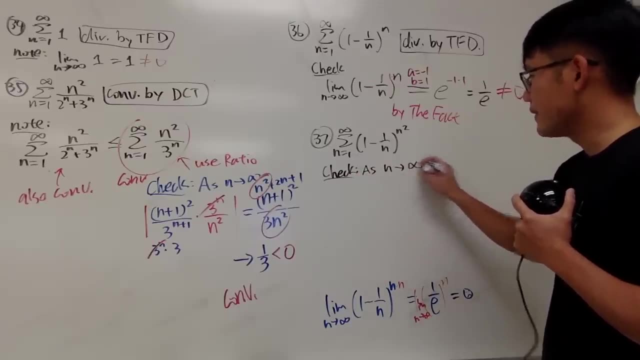 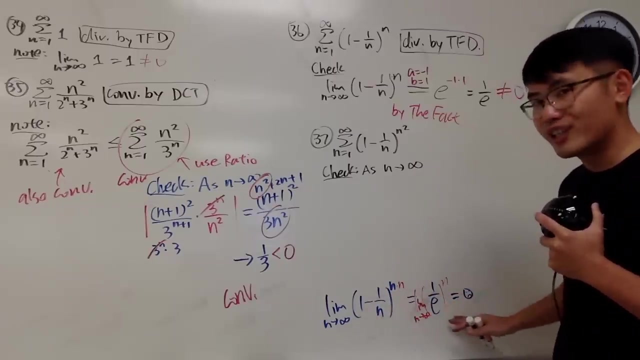 Right. So here's the deal. I'll just tell you guys, We are going to check as n goes to infinity Again. the purpose of doing this now is the root test- Right, Because the test for divergence, it wouldn't work. 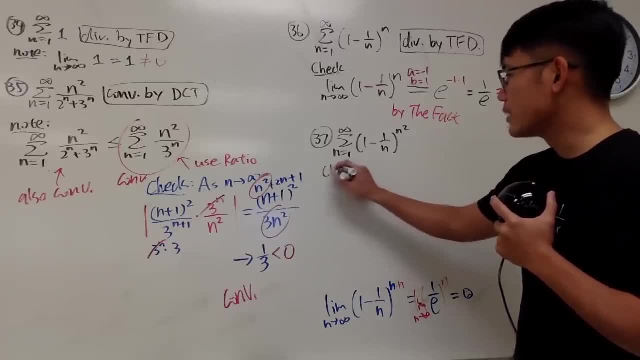 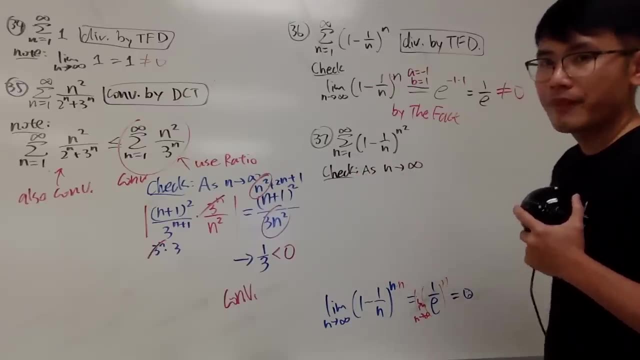 So here's the deal. I'll just tell you, guys, we are going to check as n goes to infinity Again. the purpose of doing this now is the root test right, Because the test for divergence it wouldn't work. 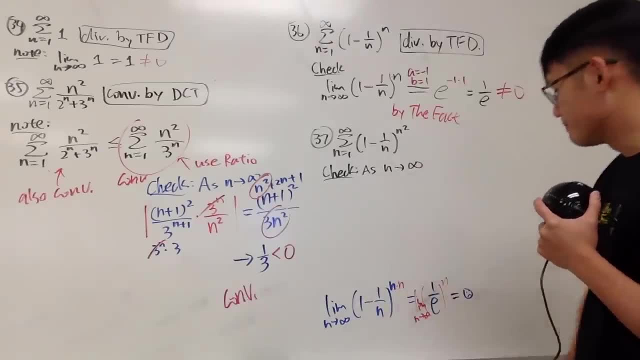 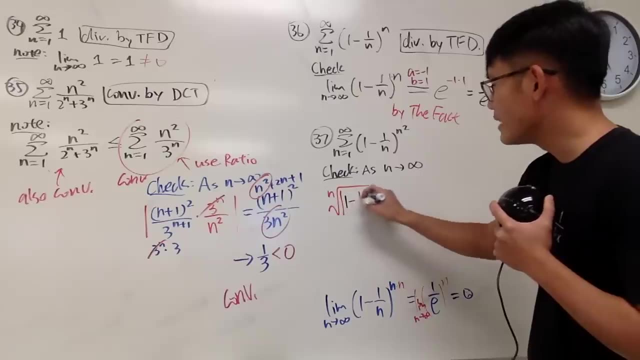 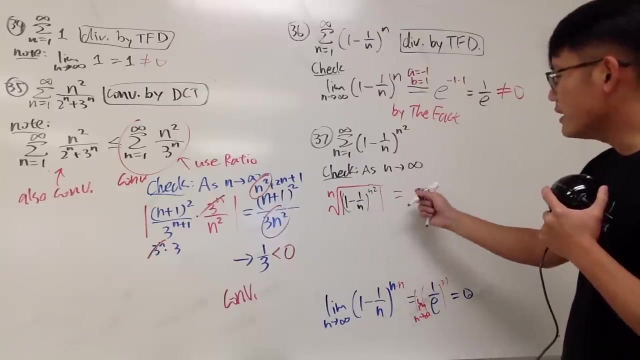 This right here, a n does approach 0.. All right, root test. in actual, you take the n's root with the absolute value and inside is 1 minus 1 over n and you have this to the n squared power like this. And now look at this part. 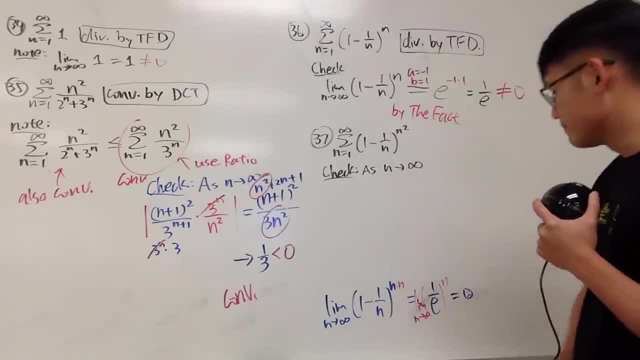 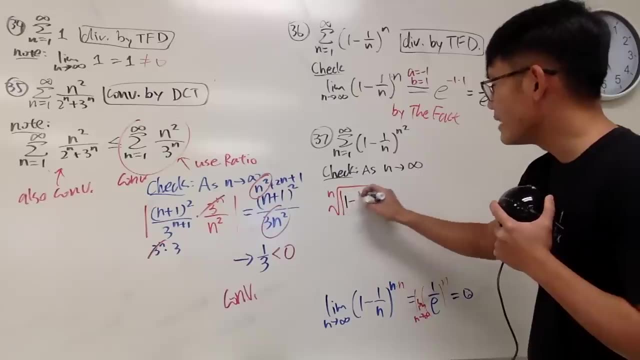 This right: here, a n does approach 0.. All right, Root test. In actual, you take the nth root with the absolute value and inside is 1 minus 1 over n And you have this to the n square power like this: 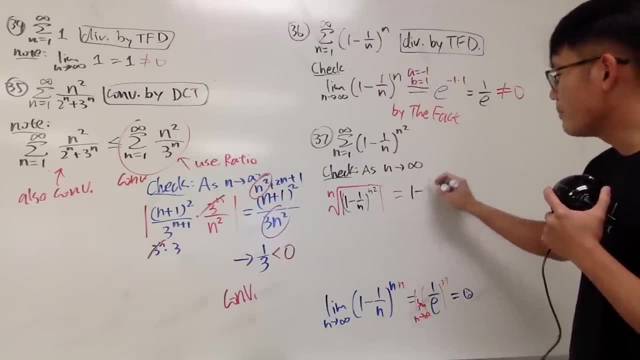 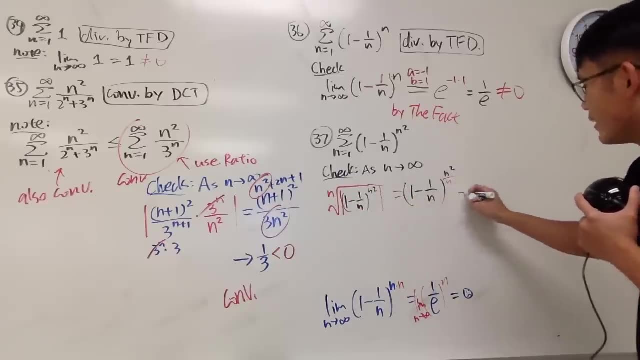 And now look at this part. This is the same as saying 1 minus 1 over n. You have n square and you have to divide it by n for the index And through the algebra you see this is 1 minus 1 over n. 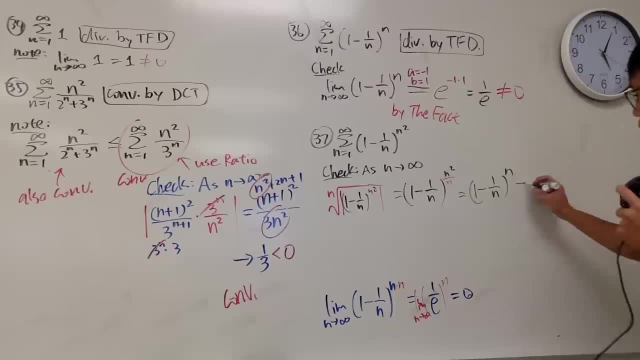 raised to the nth power And check this out. This right here we know a is negative, 1 and b is 1.. So let me just indicate that, So you can see. I'm using the fact right here And in this case, 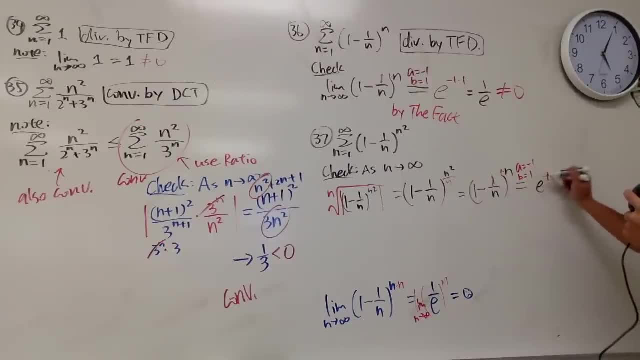 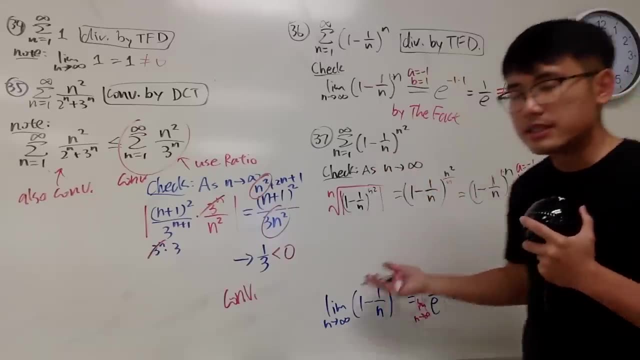 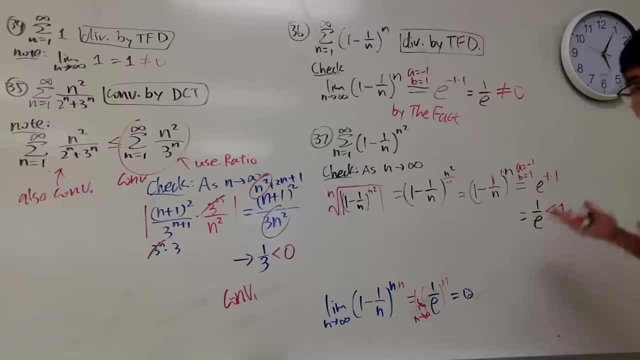 we get e to the negative 1 times 1.. And of course, this is the same as saying 1 over e. Now, because this is from the root test and we get the limit is 1, which is 1 over e, which is less than 1.. 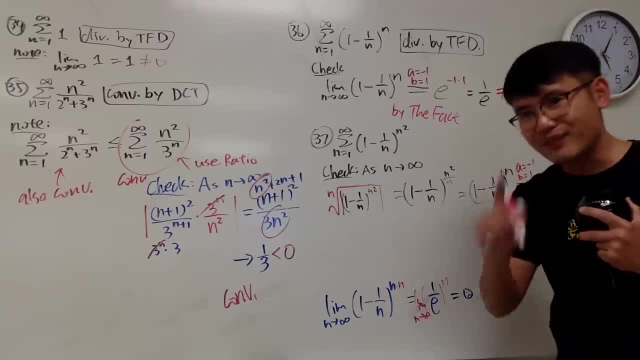 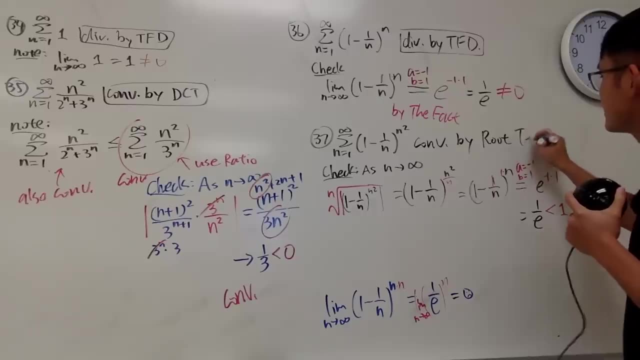 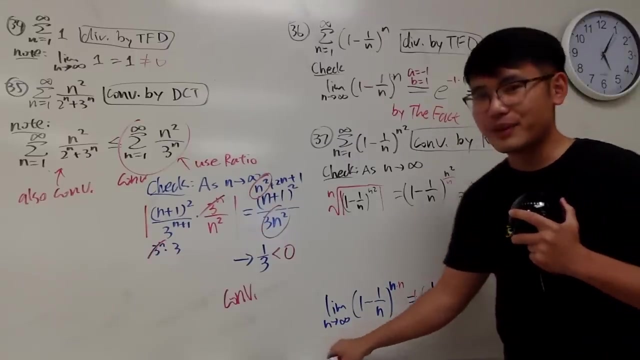 This right here does tell us that this right here converges. This right here converges by the root test Right. So please be sure that you study all these things carefully, Know the difference here and there, and all the good things Right. 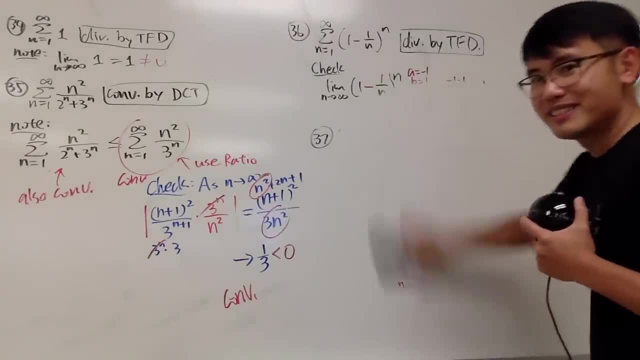 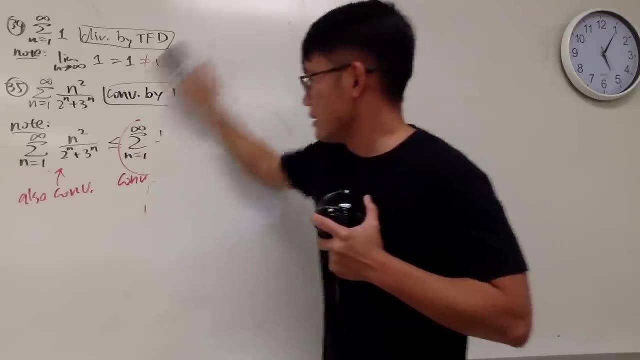 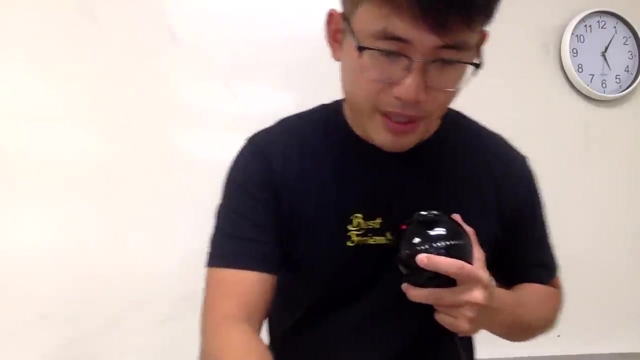 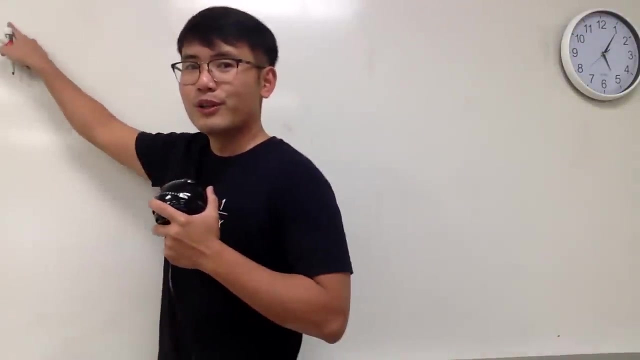 Okay, So that was number 37. And now let's see: Hmm, Okay, Number 38. It's like another page done, It feels so good. Number 38. Here we are going to do the sum from 1 to infinity. 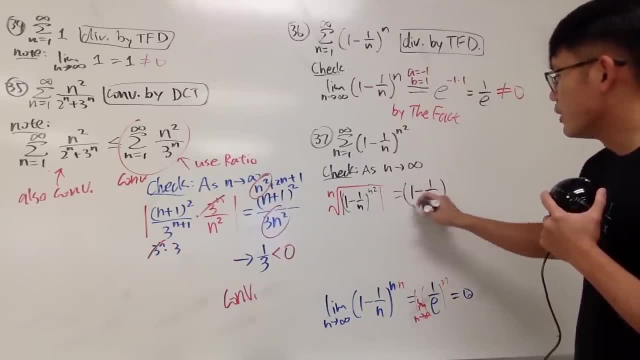 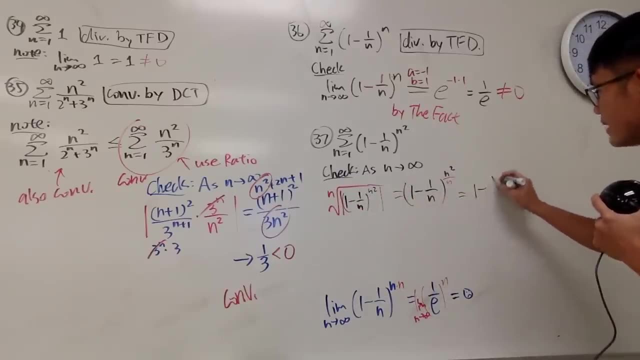 This is the same as saying 1 minus 1 over n. You have n squared and you have to divide it by n for the index And through the algebra you see this is 1 minus 1 over n raised to the n's power. and check this out. 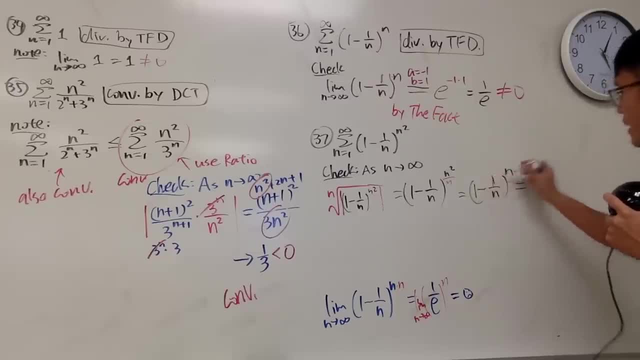 This right here. we know a is negative 1 and b is 1.. So let me just indicate that So you can see. I'm using the fact right here and in this case we get e to the negative 1 times 1, and of course this is the same as saying 1 over e. 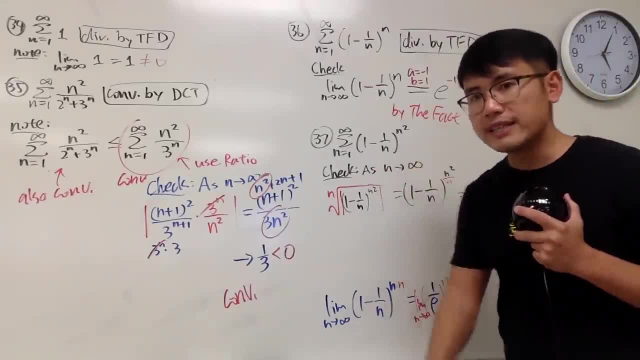 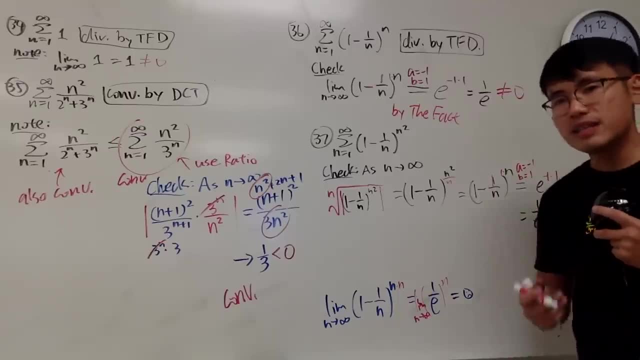 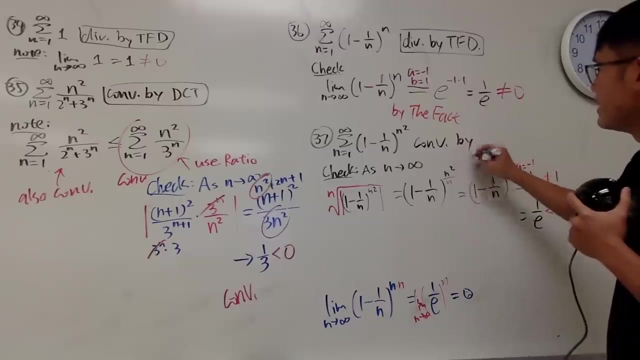 Now, because this is from the root test and we get: the limit is 1 over e, which is less than 1, this right here does tell us that this right here converges. This right here converges by the root test. 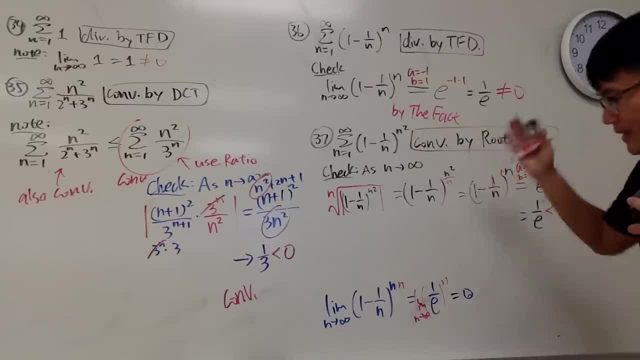 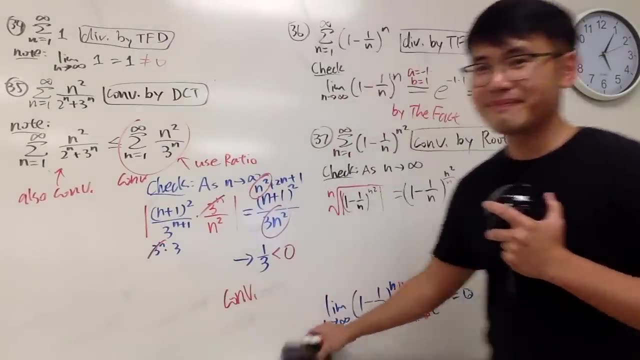 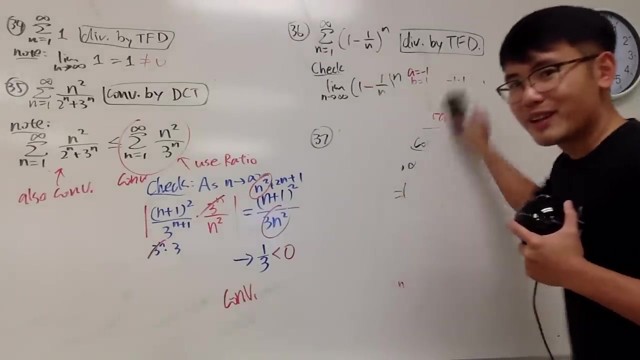 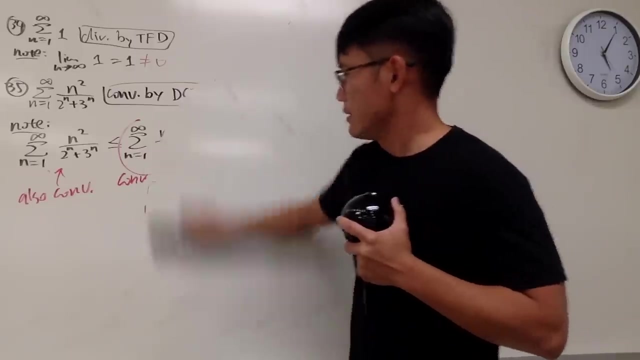 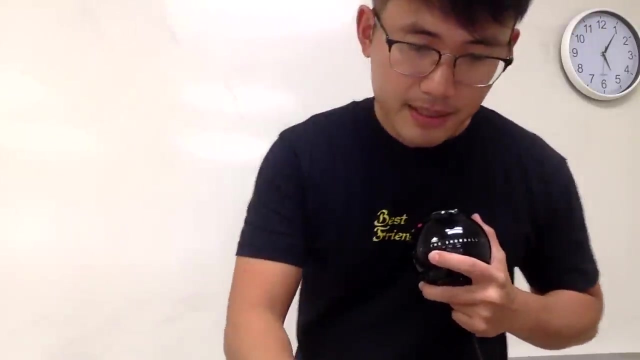 Alright. So please be sure that you study all these things carefully, Know the difference here and there, and all the good things, Alright, Okay, so that was number 37, and now let's see: Hmm, Okay, number 38.. 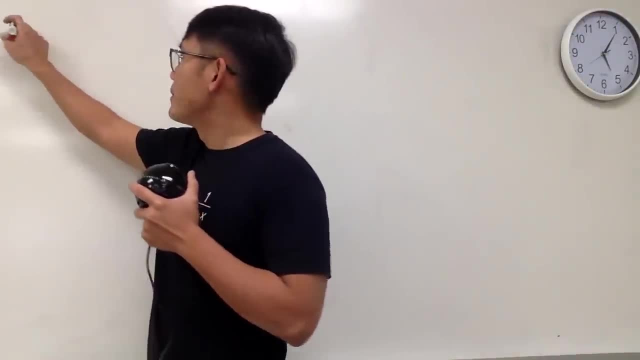 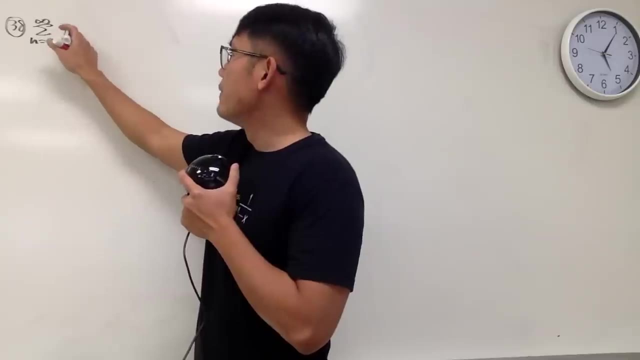 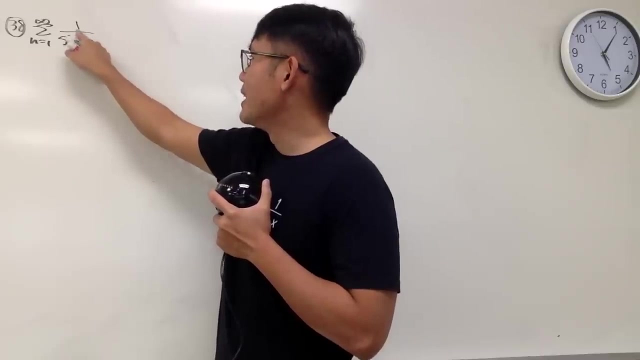 Another page done, It feels so good. Number 38.. Here we are going to do the sum as n goes from 1 to infinity, And here we have 1 over sine to the 4th power n, Sine to the 4th power n. 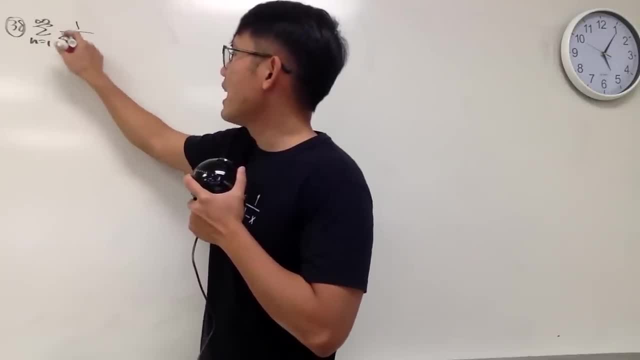 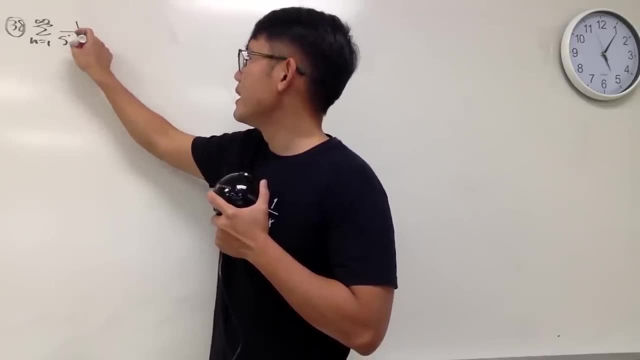 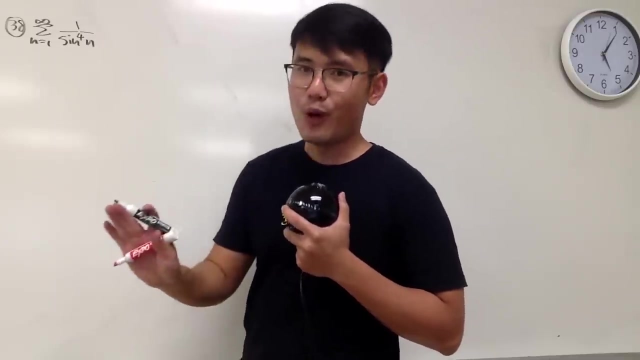 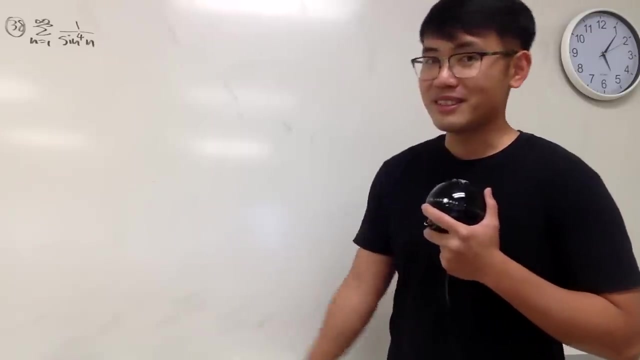 And here we have: 1 over sine to the fourth power n, Sine to the fourth power n. Hmm, Does a? n go to 0?? No, Sine. the limit for sine as x or n go to infinity just does not exist. 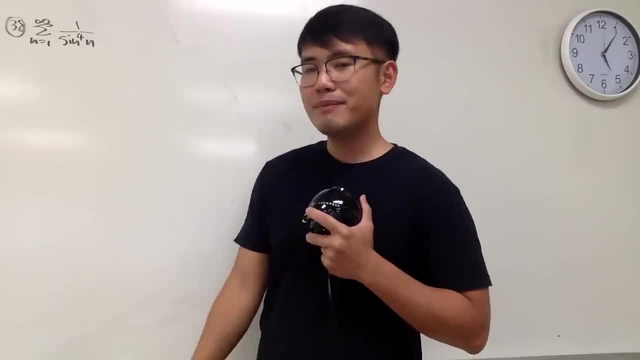 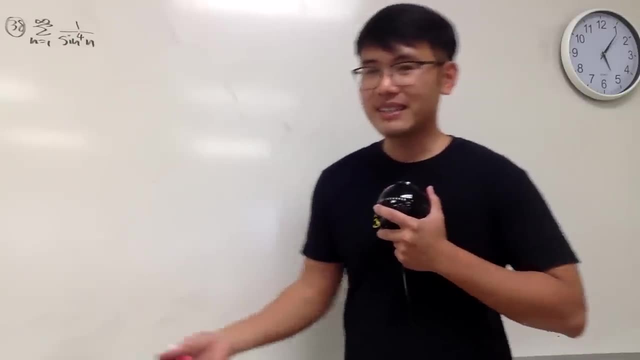 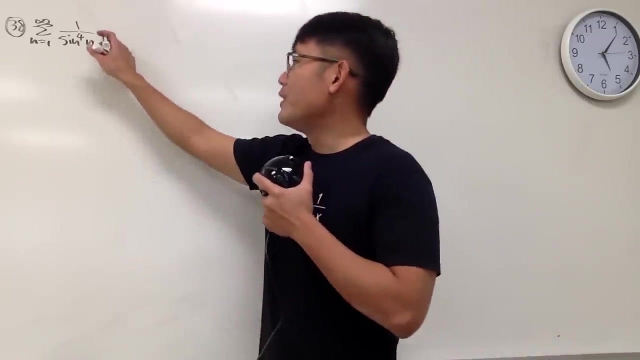 Hmm, Does a? n go to 0?? No, Sine, the limit for sine as x will n go to infinity just does not exist. We have the 4th power still? No, This right here, Very easy Diverges by test. 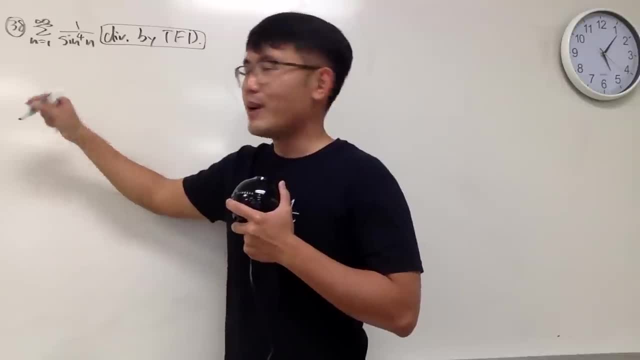 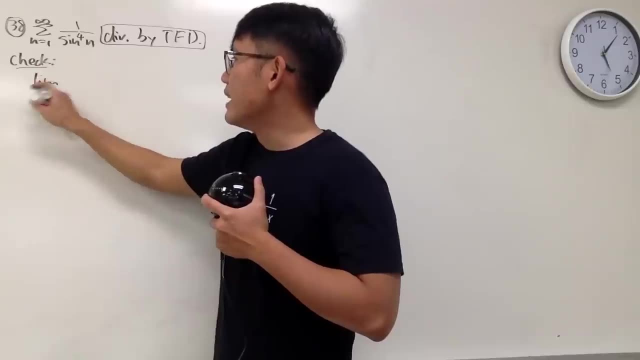 For divergence. That's it. So I'll just tell you guys that if you check the limit again, this is for the test for divergence. the limit as n goes to infinity of 1 over sine to the 4th power n This right here, seriously. 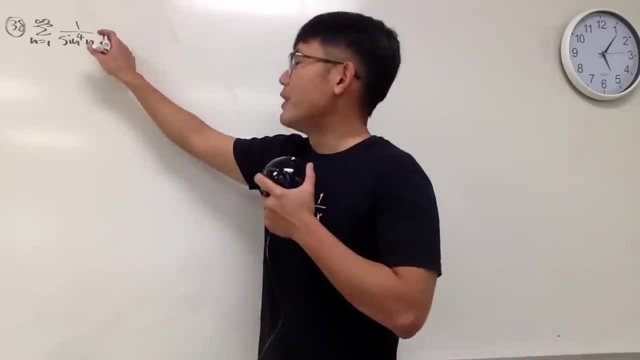 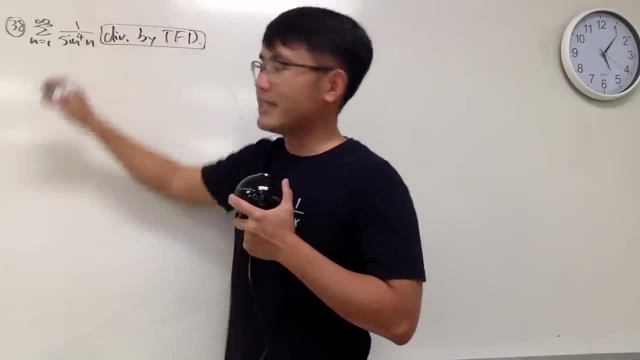 when you have the fourth power. still, This right here very easy Diverges by test for divergence. That's it. So I'll just tell you guys that if you check the limit again, this is for the test for divergence. 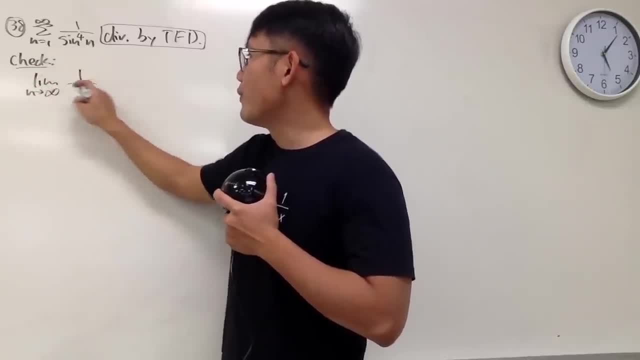 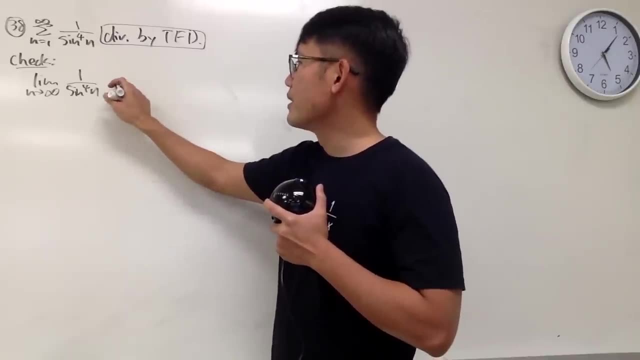 the limit, as n goes to infinity, of 1 over sine to the fourth power n this right here, seriously, you just go up and down, up and down, right? So this right here does not exist. Technically this does not exist. 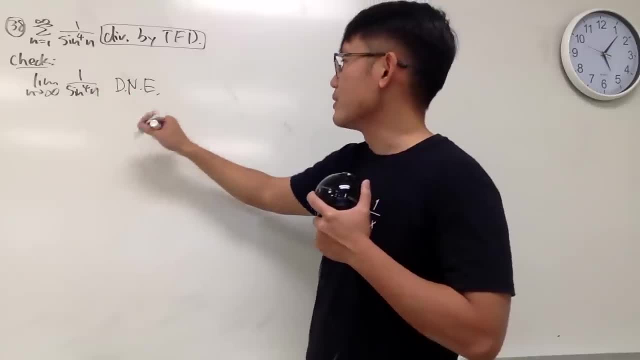 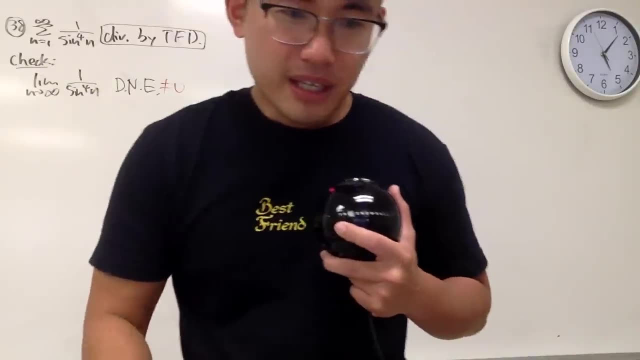 The bottom doesn't even go to infinity, so it's not approaching 0.. And it does not exist means it's not 0.. So test for divergence, That's it, Okay. Now let's look at another famous one. 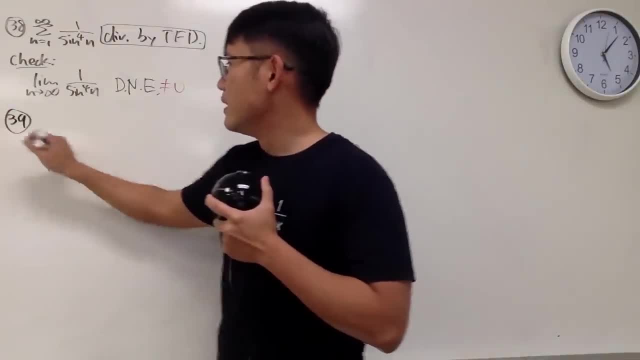 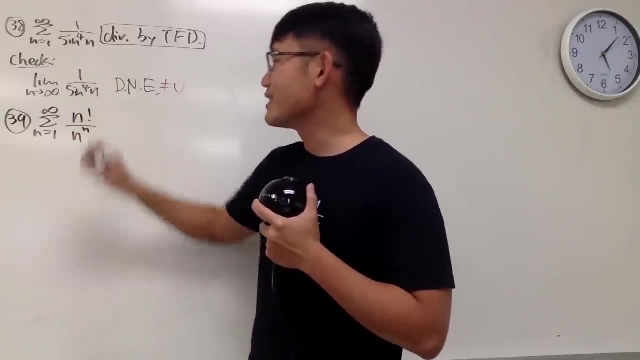 number 39.. So the sum as n goes from 1 to infinity, and here we have n factorial over n to the nth power, And this is the example I will demonstrate in my class all the time. Okay, Yes, Ratio test. 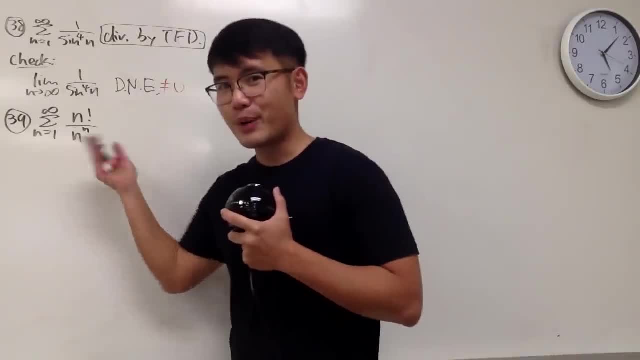 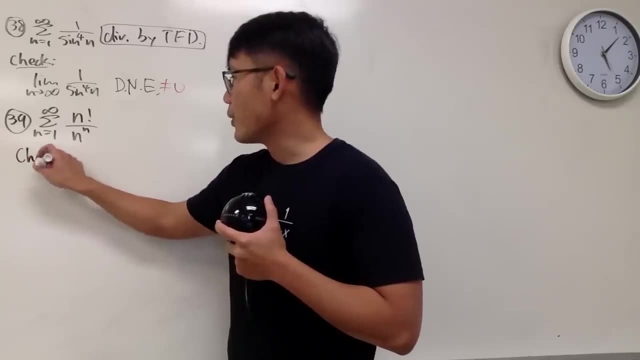 Very good Factorial and also the power in the n right, n in the power, sorry. And then here we go. So I will just go ahead and tell you we're going to check as n goes to infinity. 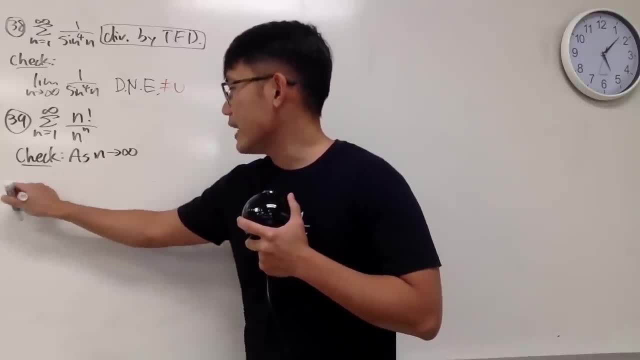 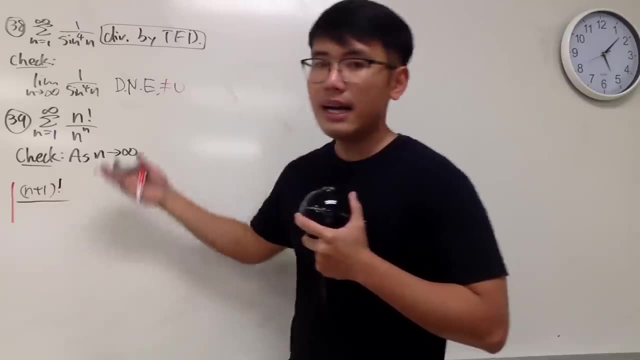 well, put the n plus 1 into all that. so we have the absolute value, n plus 1 factorial, and we divide it by. on the bottom, here we have n plus 1 raised to the n plus 1 power and we multiply by. 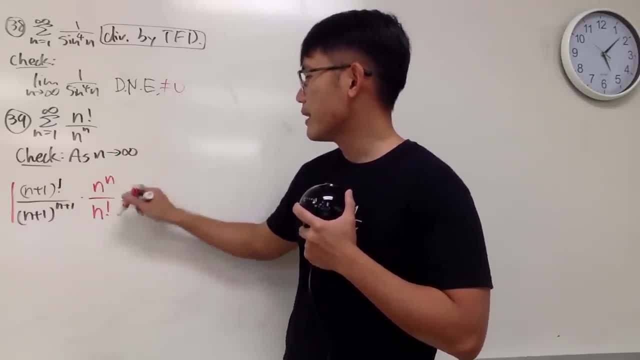 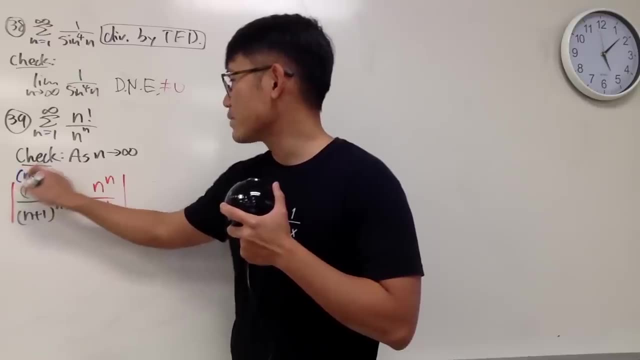 n to the n over n factorial. So that's the usual thing. Now we are going to cancel things out. Well, here it's nice. This is just n plus 1 times n factorial. This and that cancel out. 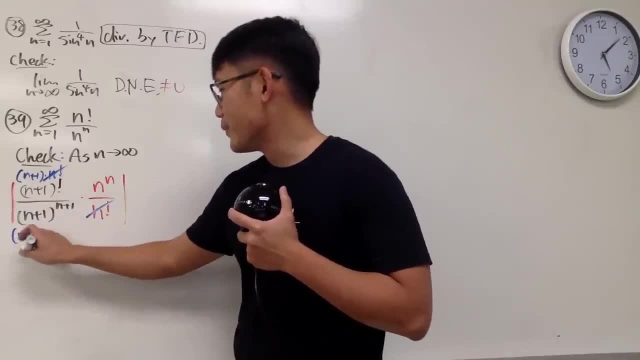 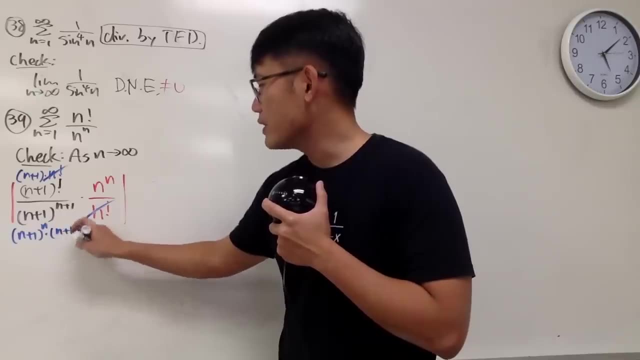 Ah, cannot, okay, okay, okay, I see that this is before I complain. this is what we can do. This is n plus 1 to the nth power times, n plus 1 to the first power. and look at: 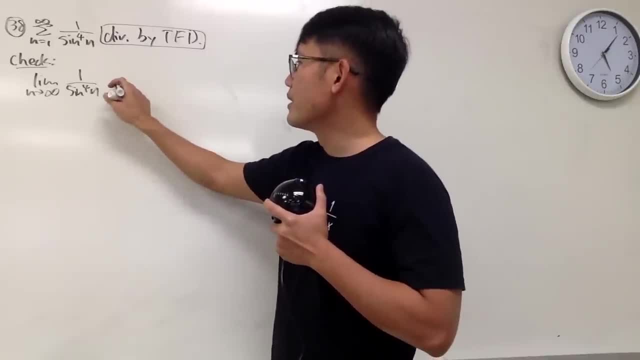 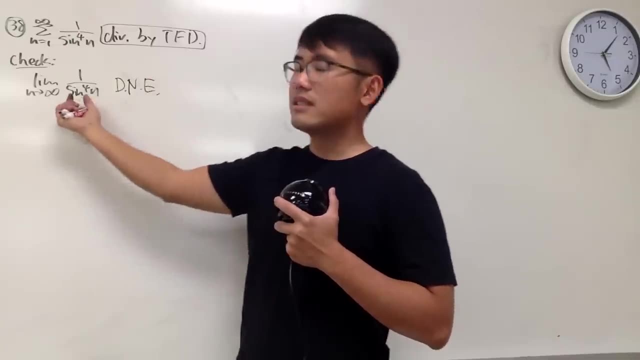 you just go up and down, up and down, right. So this right here is does not exist, Right, This right here. Technically this does not exist. The bottom doesn't even go to infinity, so it's not approaching 0.. 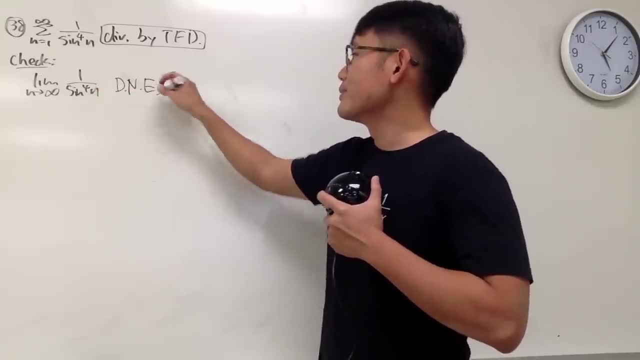 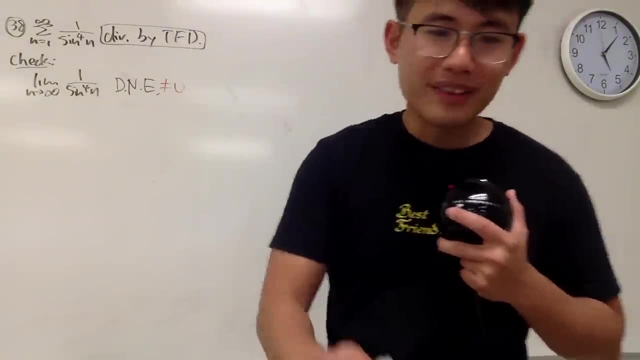 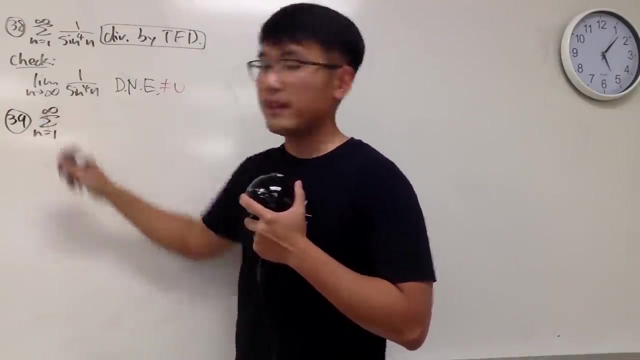 And it does not exist means it's not 0.. So test for divergence, That's it. Okay. Now let's look at another famous one, Number 39.. So the sum as n goes from 1 to infinity. 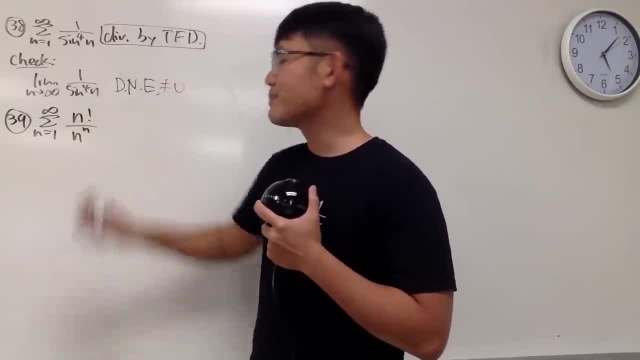 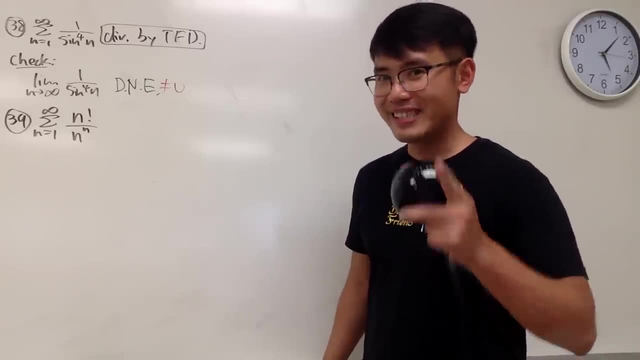 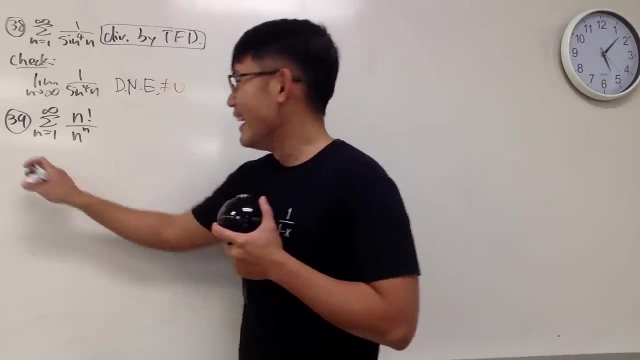 And here we have n factorial over n to the nth power, And this is the example I will demonstrate in my class all the time. Okay, Yes, Ratio test, Very good Factorial, and also the power in the n right, n in the power, Sorry. And then here we go. 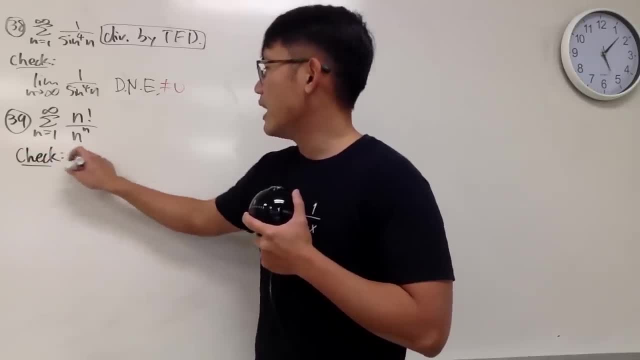 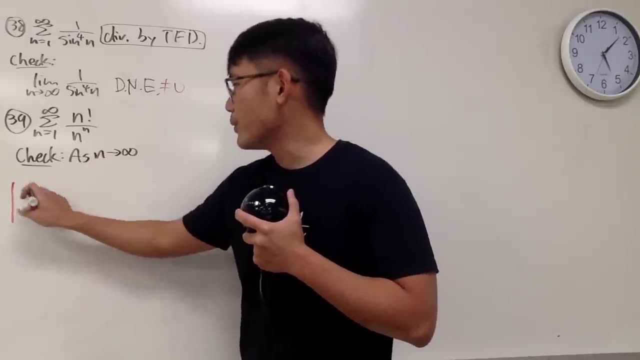 So I will just go ahead and tell you we're going to check as n goes to infinity. Well, put the n plus 1 into all that, so we have the absolute value, n plus 1 factorial, And we divide it by on the bottom. here we have n plus 1. 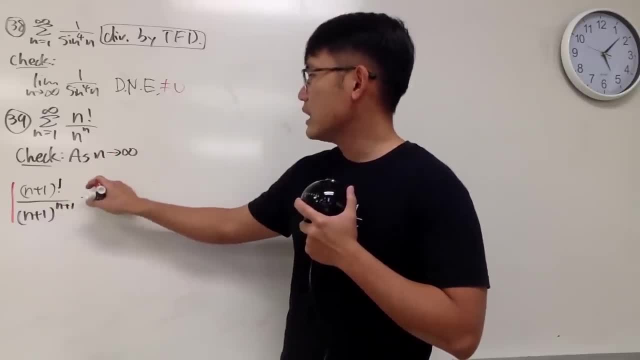 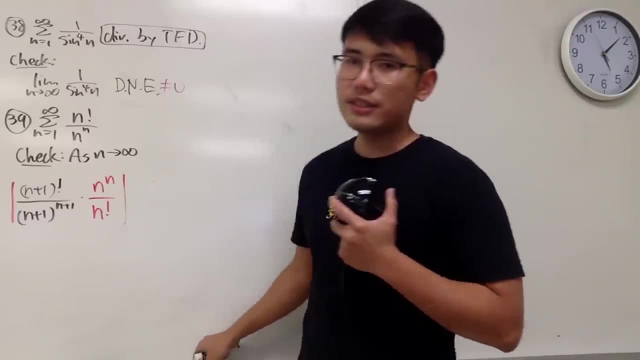 raised to the n plus 1 power and we multiply by n to the n over n factorial. So that's the usual thing. Now we're going to cancel things out. Well, here, it's nice. This is just n plus 1 times n factorial. 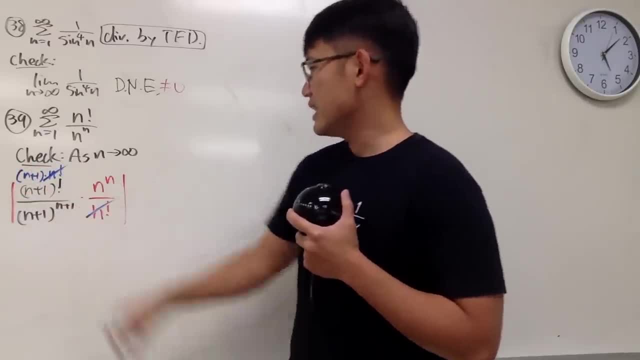 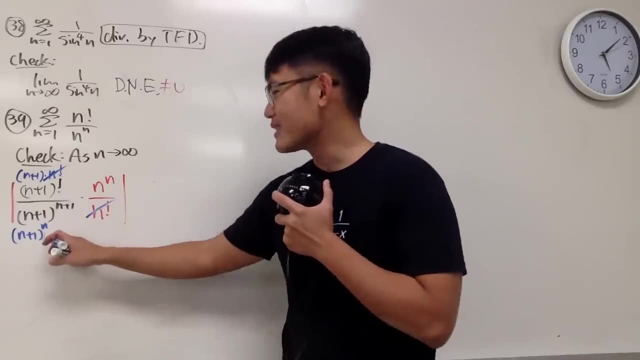 This and that. cancel out? Ugh, cannot, okay, okay, okay, okay. I see that this is. before I complain, I should look at what we can do. This is n plus 1 to the nth power times, n plus 1 to the first power. 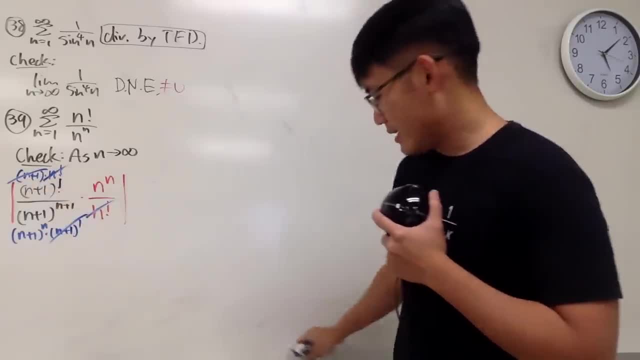 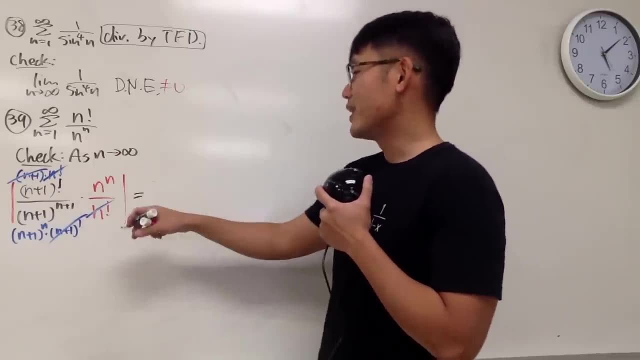 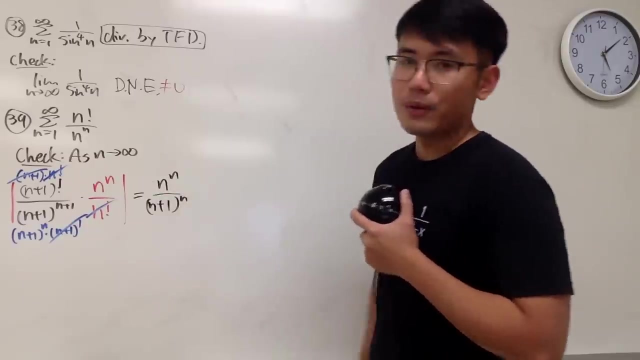 And look at this and that can be cancelled out. Huh, So now we end up with this, which is again, everything is positive. that's nice. so just look at it inside. On the top we have n to the n, on the bottom we have n plus 1 to the nth power. 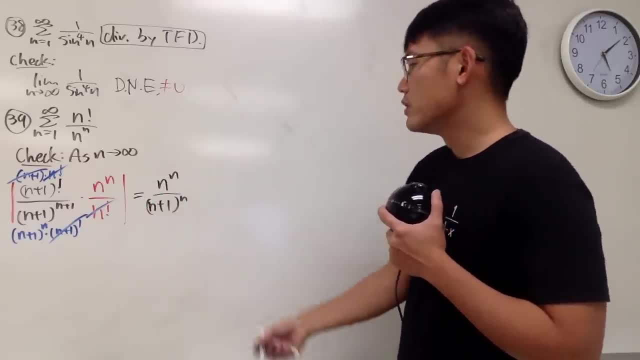 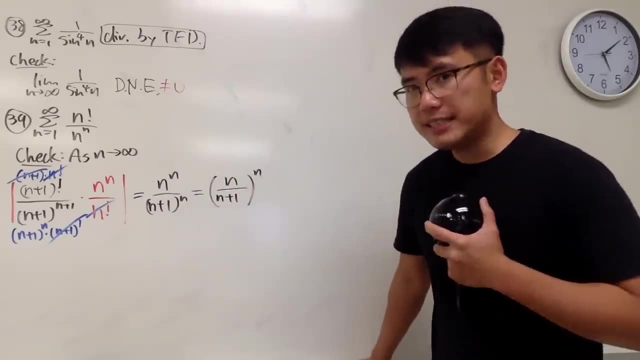 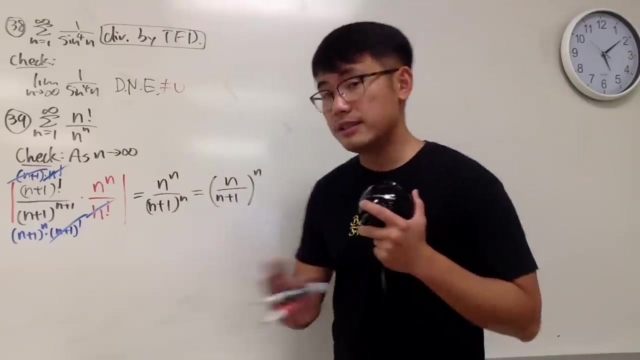 Okay, both of them are of to the nth power, so we can write this down as parentheses: n over n plus 1 raised to the nth power. Very nice, But what's this limit, though? This right here is not 1, the limit right here is not 1.. 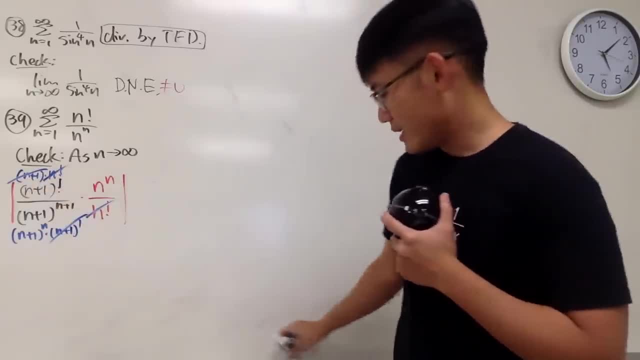 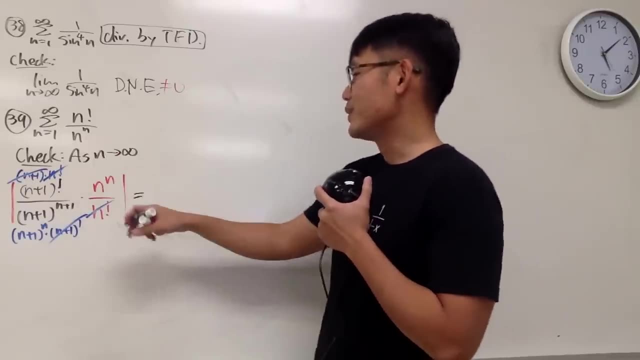 this and that can be cancelled out. huh. So now we end up with this, which is again, everything is positive. Well, that's nice. So just look at it inside. On the top, we have n to the n. 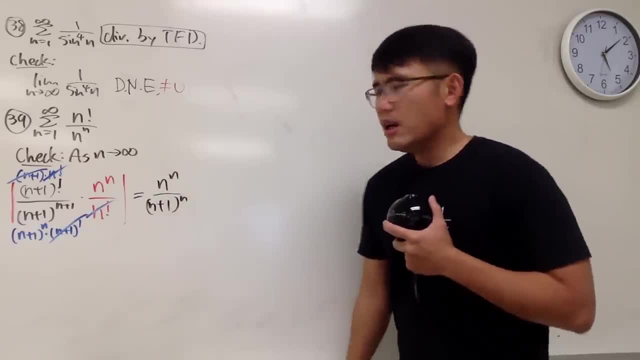 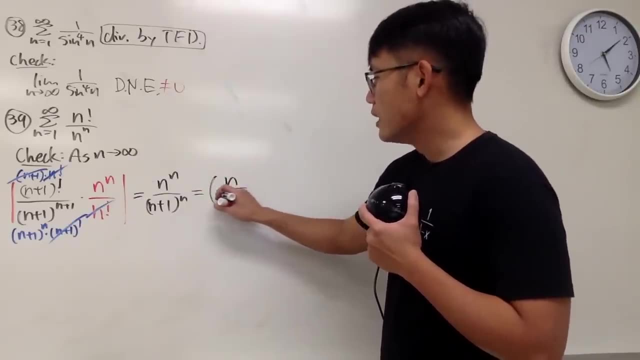 On the bottom we have n plus 1 to the nth power. Okay, both of them are of to the nth power, so we can write this down as parentheses: n over n plus 1 raised to the nth power. Very nice. 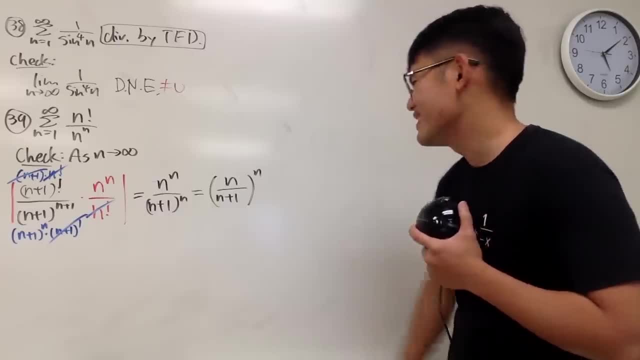 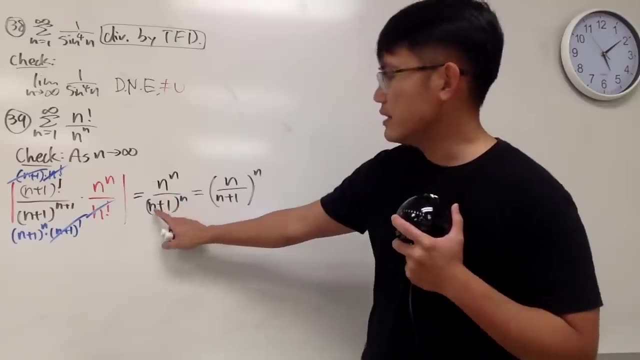 But what's this limit, though? This right here is not 1.. The limit right here is not 1.. Do not just ignore the 1 and just say this is about the same as n to the nth power, It's not 1.. 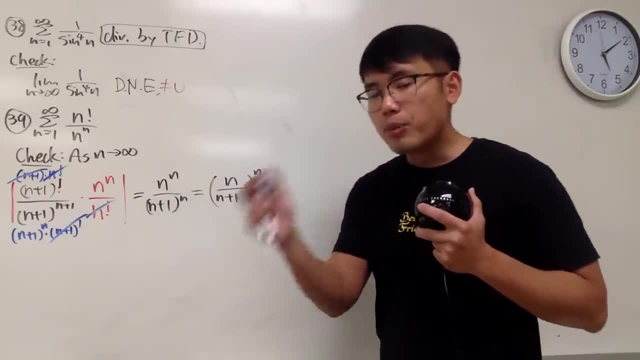 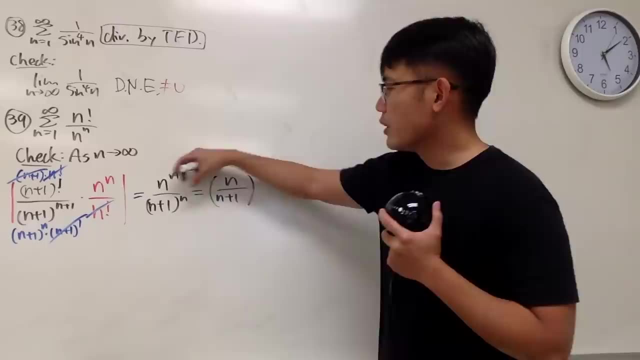 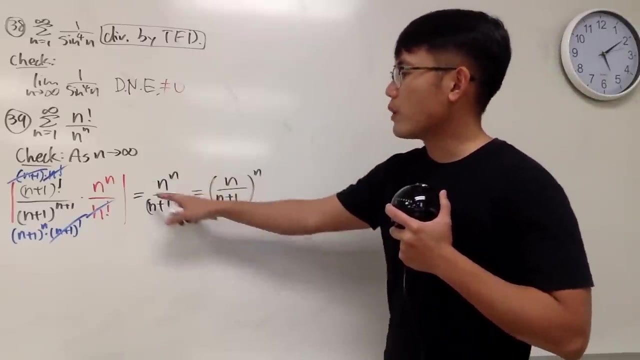 Why? Because the product of the limit is the same as the limit of the product. if you have the finite amount of product, So technically right here, you have infinitely many n to the nth power over n, plus 1 to the nth power. 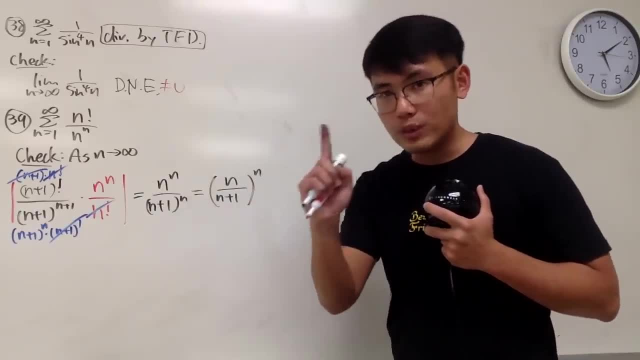 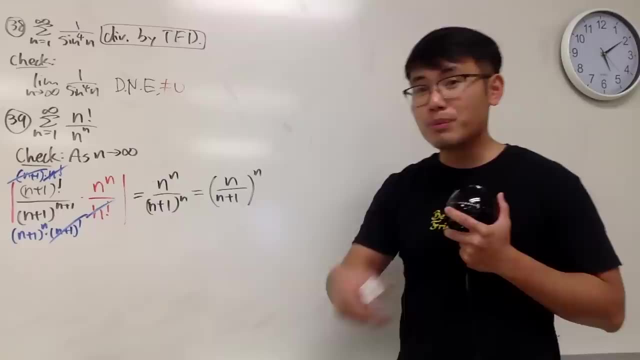 I agree with you. if you have n to the 5th power over n plus 1 to the 5th power, that would be with limit 1.. That's okay, But when n is also going to infinity, you have infinitely many. 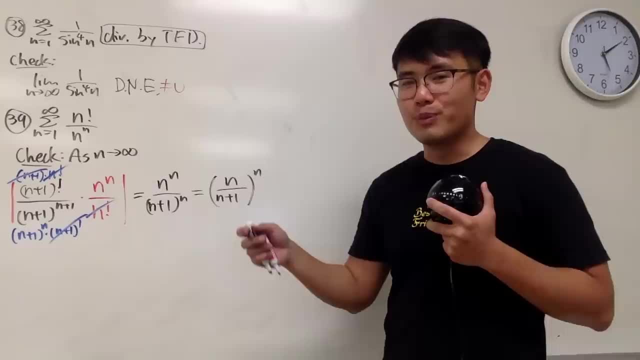 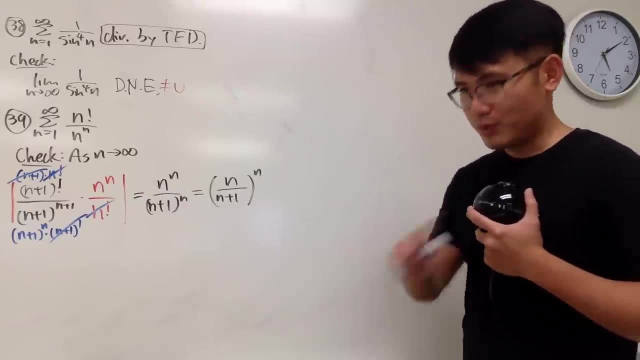 of those 1s multiplied and they are not technically 1.. They are, like you know, maybe like 1.0001 or 0.9999.. When you put on the 1, that's actually just like you know. 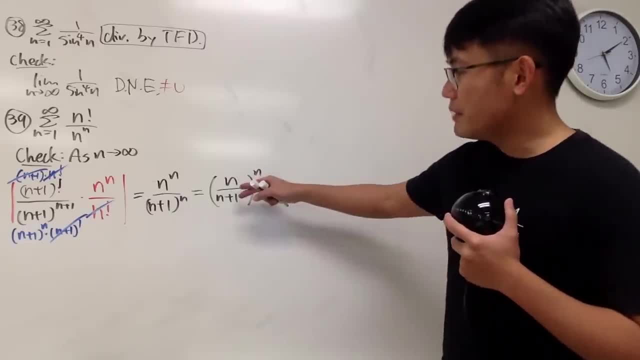 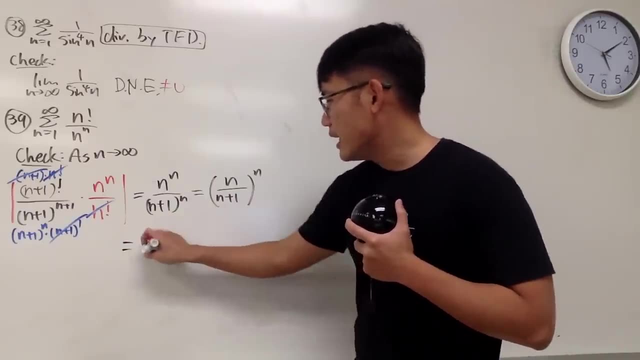 0.9999.. But here the way to do is the fact: Flip the inside, make the power negative. Let me show you. Okay. so here we go. I'm going to look at the inside as n plus 1. 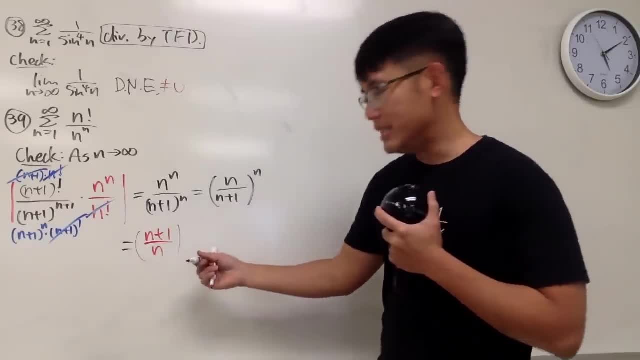 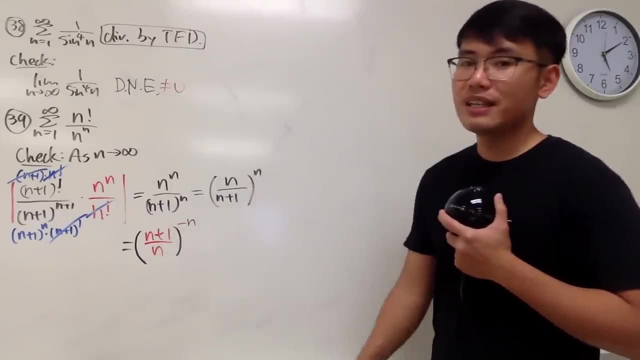 over n and in order for me to make this legal, I will have to make the power negative. So we have to have the negative n to help me out like this. And now this right here: split, split the fractions we get. 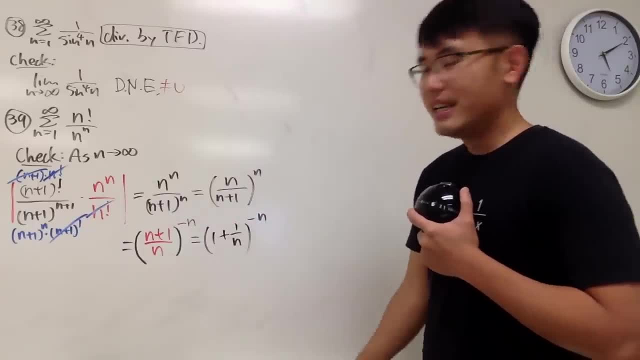 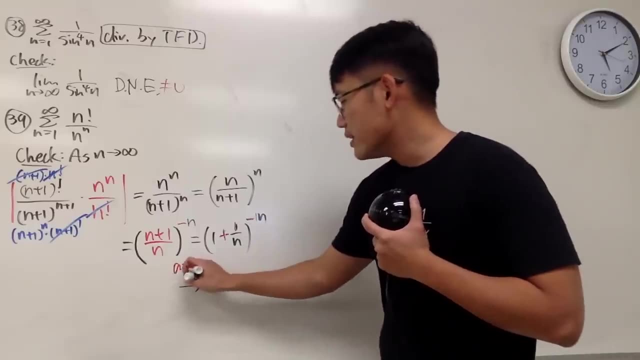 n and this is negative 1.. Like that. And now we're going to tell you: well, in this case, look here we have positive 1 but negative 1. here, a is technically positive 1 and b is negative 1. 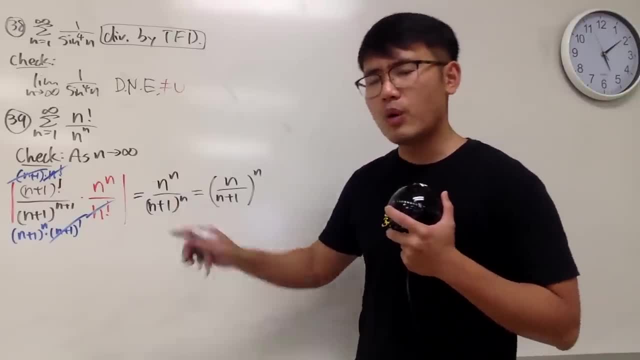 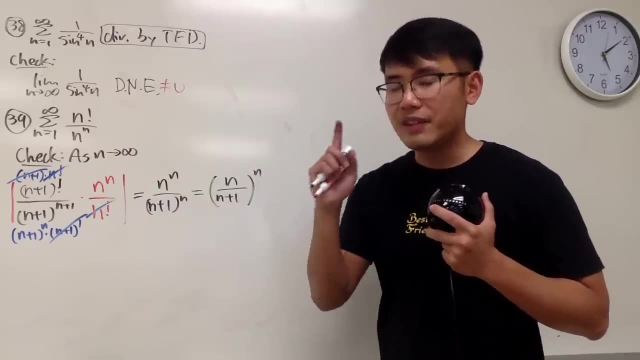 Do not just ignore the 1 and just say this is about the same as n to the nth power. it's not 1.. Why? Because the product of the limit is the same as the limit of the product if you have a finite amount of product. 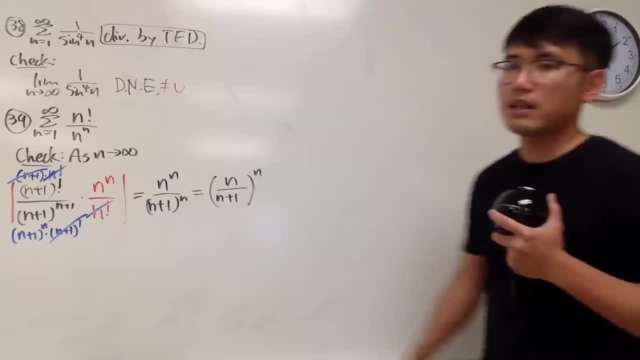 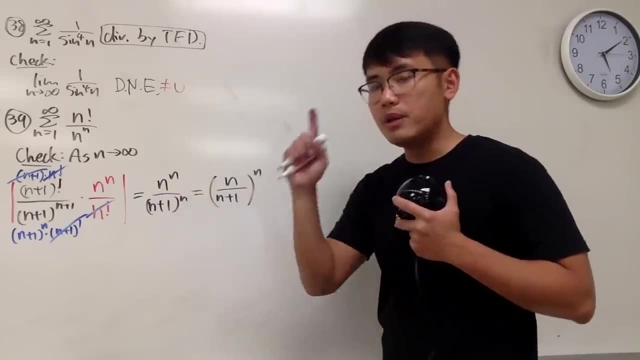 So technically right here you have infinitely many 1s multiplying. I agree with you. if you have n to the 5th power over n plus 1 to the 5th power, that would be with limit 1.. That's fine. 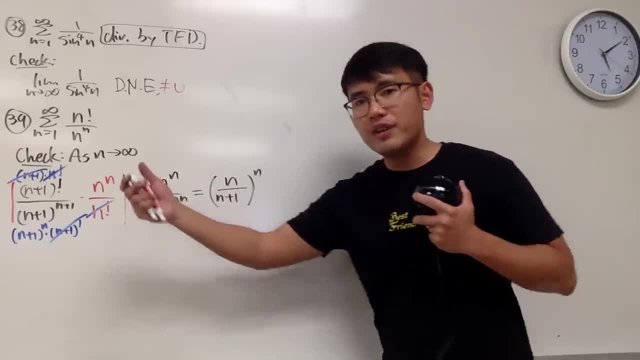 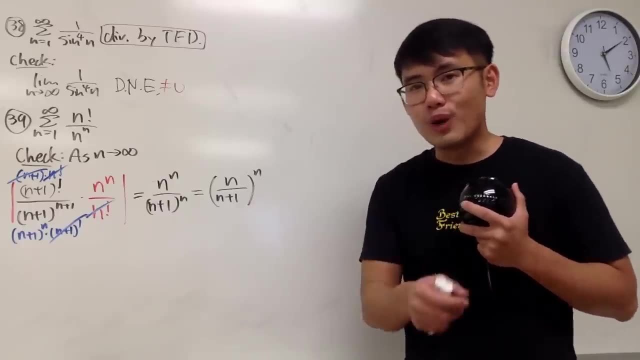 That's okay, But when n is also going to infinity, you have infinitely many of those 1s multiplied, and they are not technically 1.. They are like you know, maybe like 1.00001, or 0.999999.. 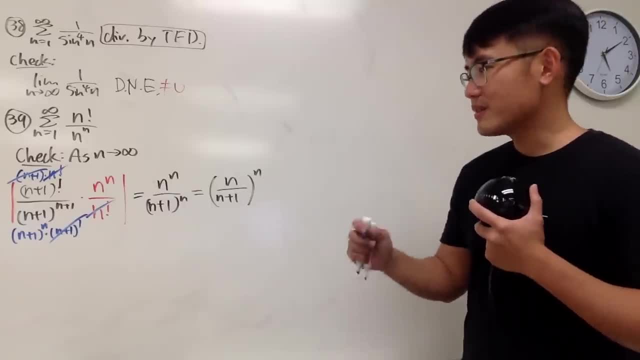 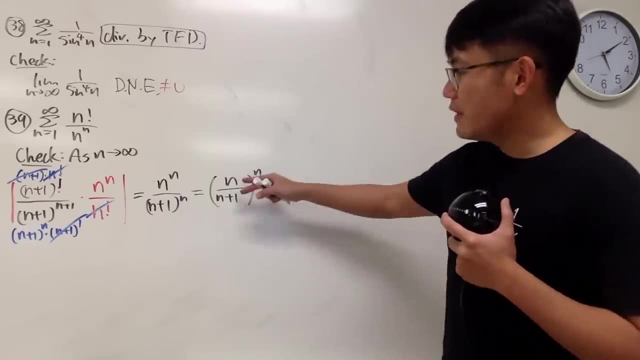 When you put on the 1, that's actually just like you know, just like that. Check them out in the video for a detailed explanation. But here the way to do it is the fact: Flip the inside, make the power negative. 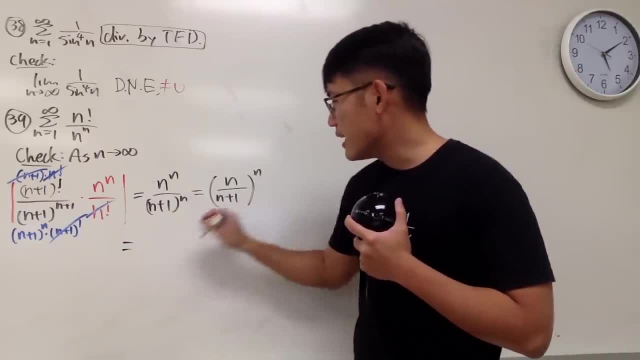 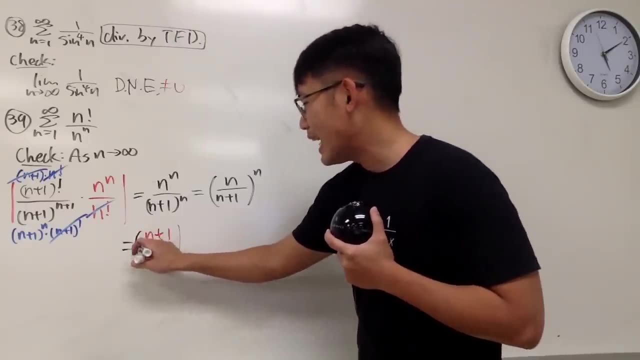 Let me show you. Okay. so here we go. We're going to look at the inside as n plus 1 over n, and in order for me to make this legal, I will have to make the power negative. So we have to have the negative n to help me out, like this: 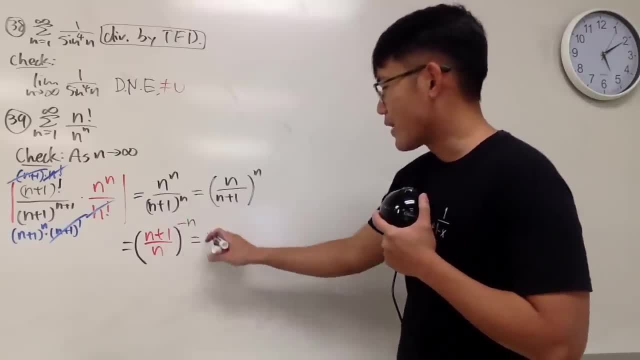 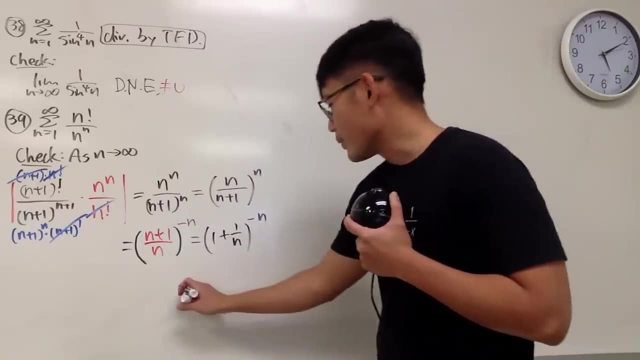 And now this right here: split the fractions, we get 1 plus 1 over n, and this is negative 1, like that. And now we're going to tell you: well, in this case, look here, we have positive 1, but negative 1 here. 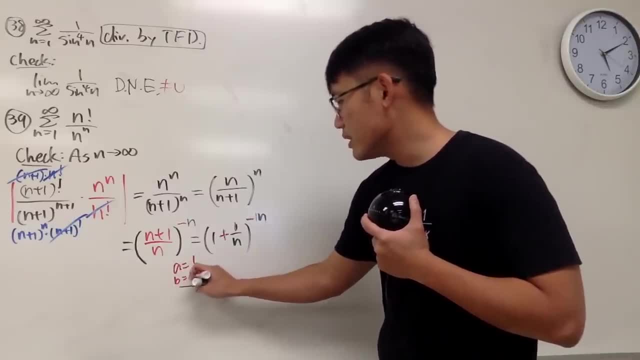 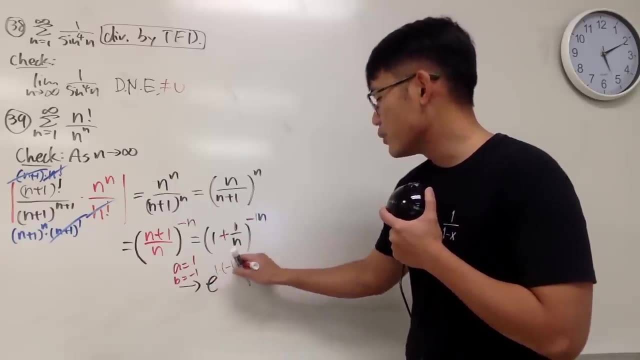 Okay, So a is technically positive 1, and b is negative 1, and we're using the fact, And when you put this down you know you're using the fact. so this is good, And you have e to the 1 times negative 1,, which is 1 over e. 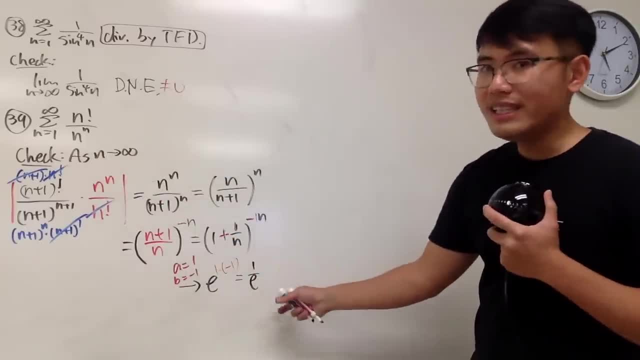 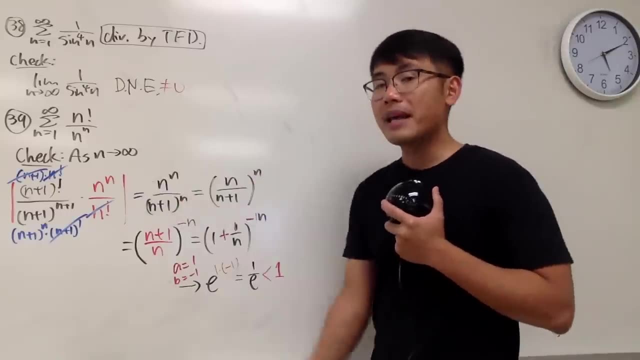 And you see the limit is approaching: 1 over e. 1 over e because e is about 2.7 or something, so this is less than 1.. That means you can come back here and say this right here: actually converges. 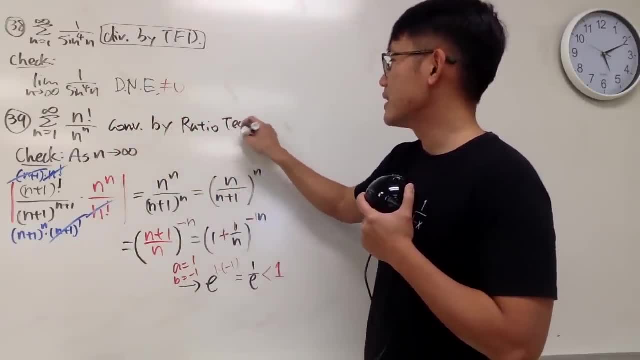 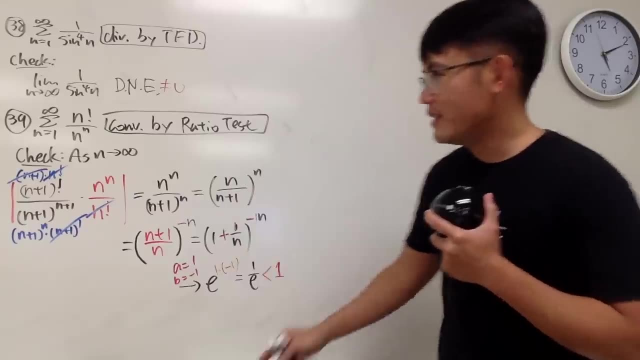 Why By the ratio. So we're going to do the test. Woo, Right, I can kind of tell that the market is about to run up, but hopefully another like 30 more questions. I don't know, though, so we'll see. 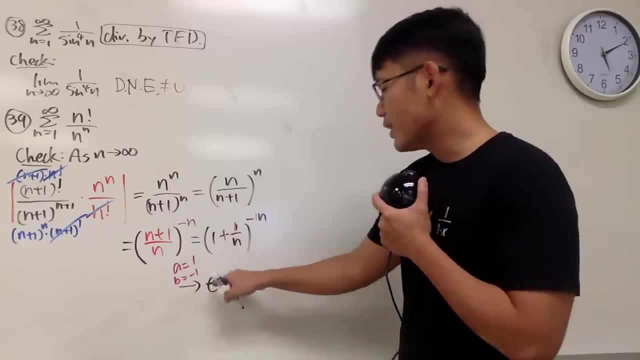 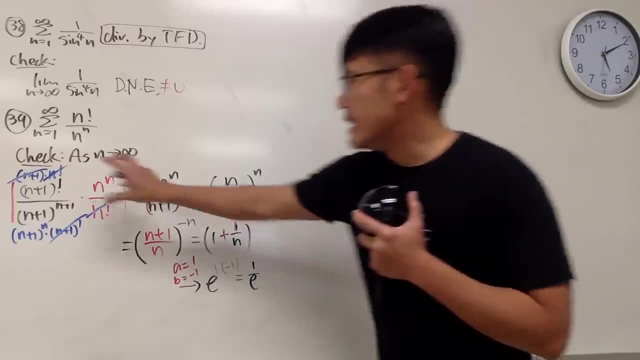 and we're using the fact, And when you put this down, I know you're using the fact. so this is good, And you have e to the 1 times negative 1, which is 1 over e, And you see the limit is approaching. 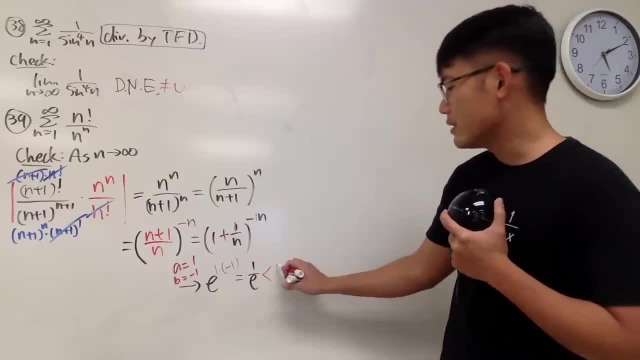 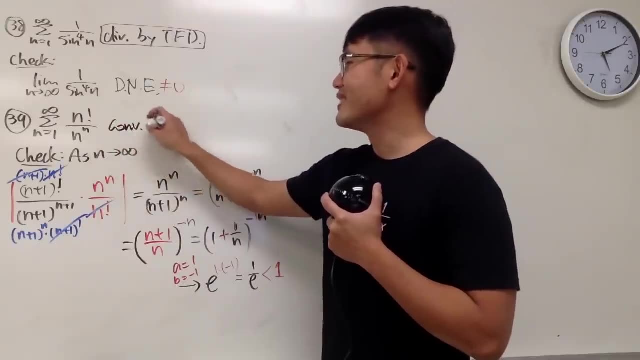 1 over e, 1 over e, which is about 2.7 or something. So this is less than 1.. That means you can come back here and say this right here: actually converges y by the ratio test. Whew. 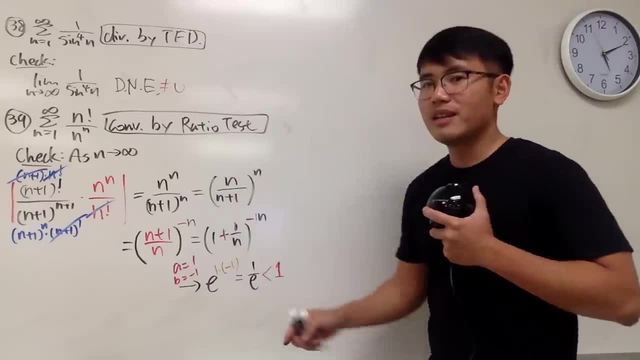 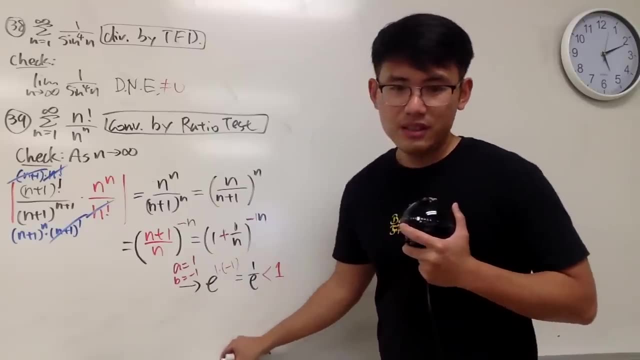 Right, I can kind of tell that the market's about to run out of ink, But hopefully another like 30 more questions. I don't know, though, so we'll see. Whew, We'll see, we'll see, we will see. 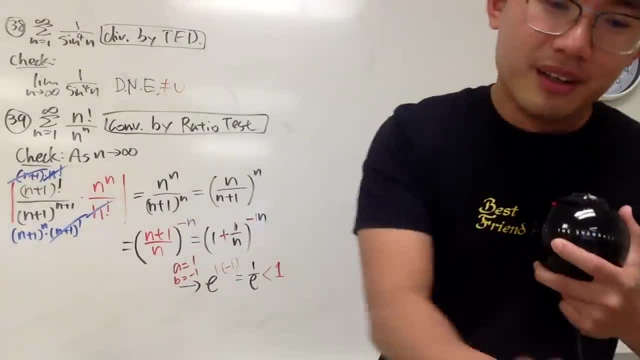 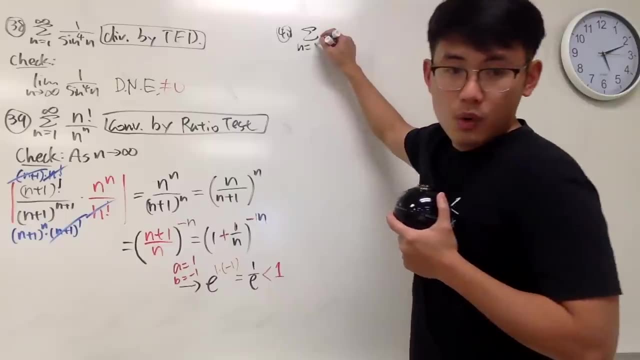 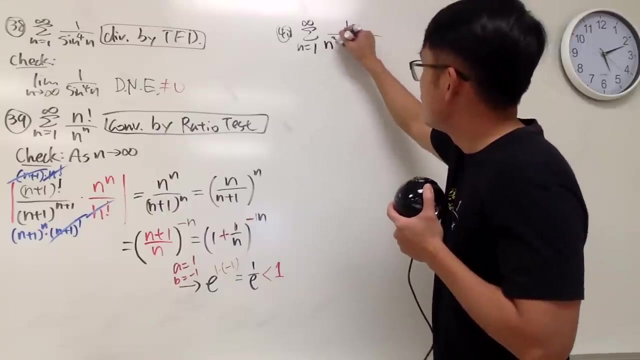 All right, Number 40. I also gave myself a big question. Let's see Number 40. We are going to look at the sum as n goes from 1 to infinity and then we have 1 over and here we have n cubed. 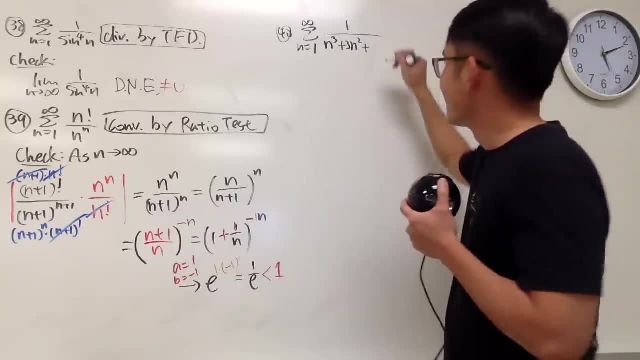 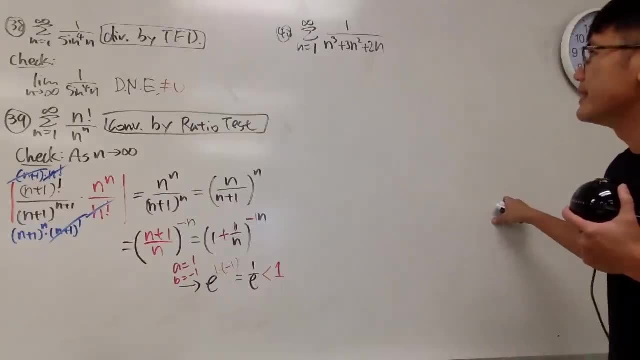 plus 3n, squared plus 2n, like this, And you know this is number 40, so we are going to actually calculate the sum. All right, It actually converges. It's 1 over n to the third power, so you can just. 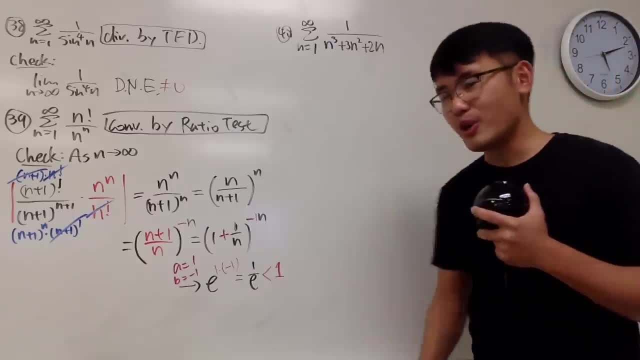 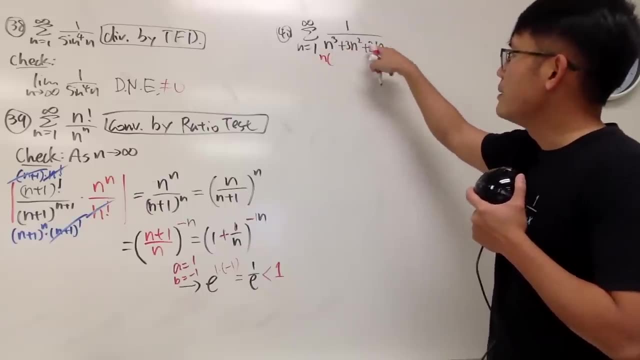 do some comparison. you know it converges. but converges to what? Let me show you. Let me factor out the denominators. I will factor out the n, so it becomes n squared plus 3n plus 2. so we can do that like: do more right. 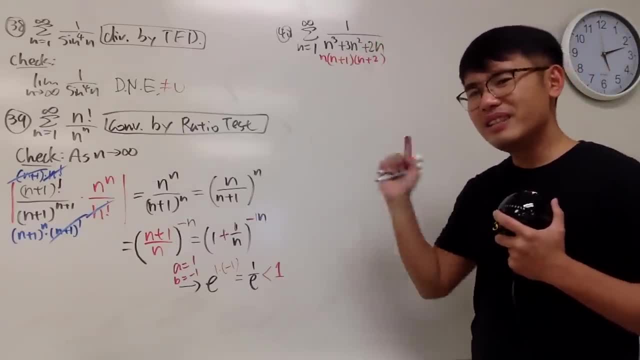 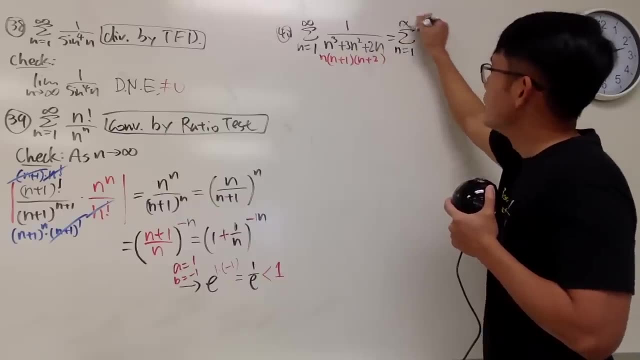 So this is n plus 1 times n plus 2.. Technically, this right here is also going to be a telescoping series. Let me show you, And to do that we are going to go fractions. You have three things on the bottom. 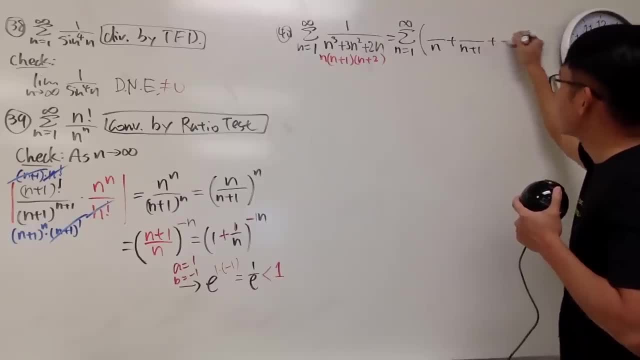 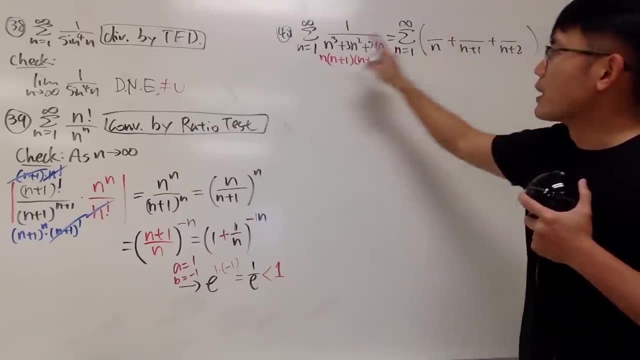 It's not that bad at all. It's the same thing. Cover up, Cover up, Cover up. All right, So here we go To figure out this number. I will come back here and I will cover up this right here. and how can I make that? 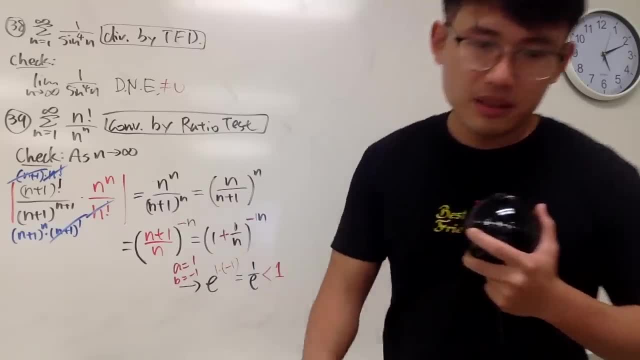 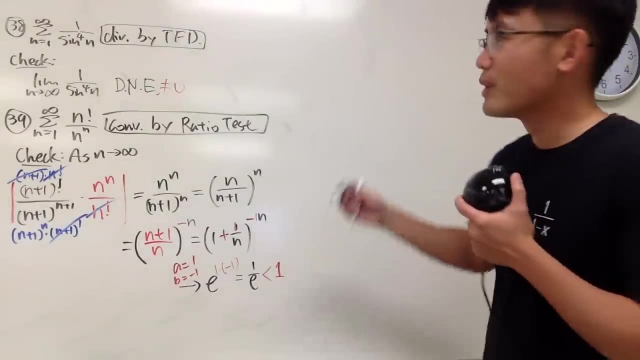 Woo, We'll see, we'll see, we will see. All right, Number 40, I also gave myself a big question. Let's see Number 40, we are going to look at the sum as n goes from 1 to infinity. 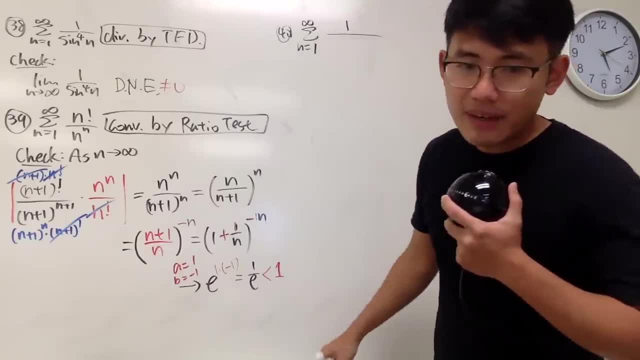 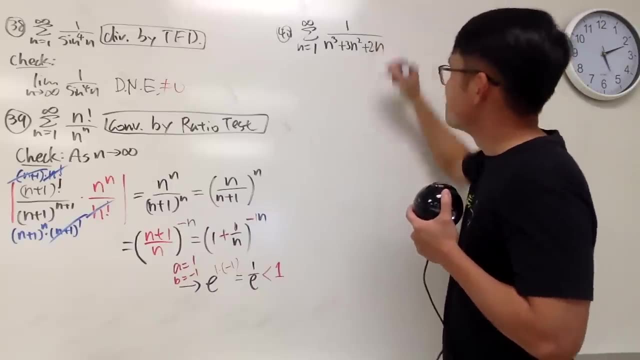 Okay, Okay. And then we have 1 over, and here we have n cubed plus 3n squared plus 2n, like this: And you know, this is number 40, so we are going to actually calculate the sum. 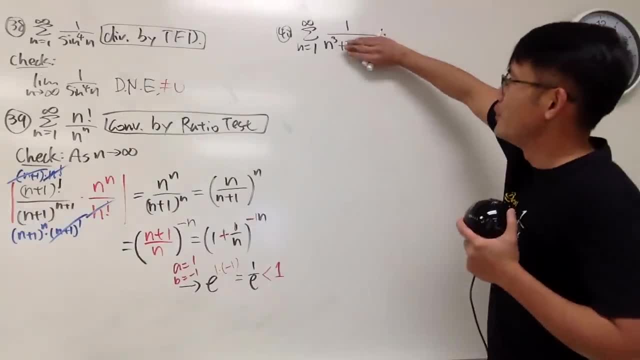 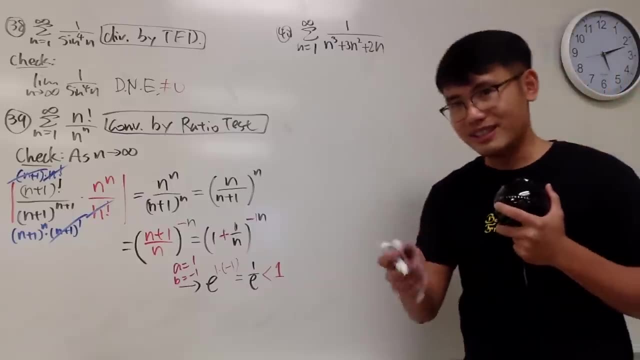 All right, It actually converges. Okay, if you cover this, it's 1 over n to the third power, so you can just do some comparison. You know it converges, but converges to what? Let me show you. 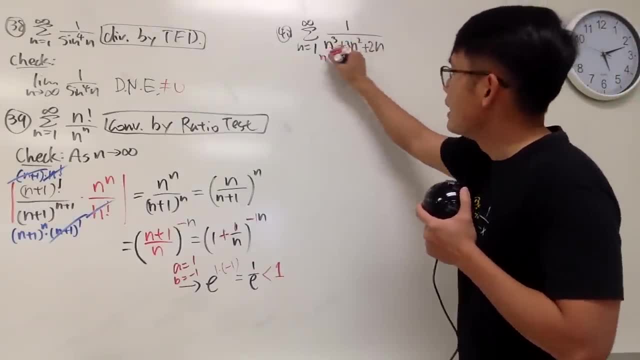 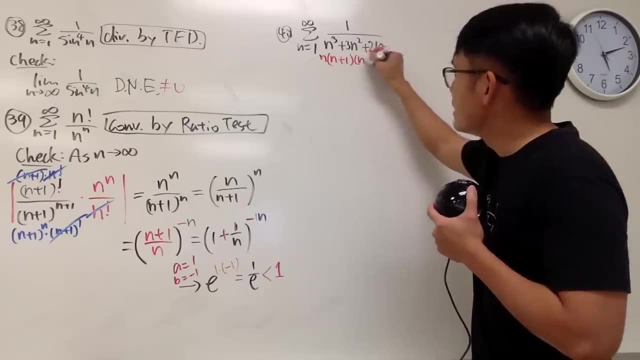 Let me factor out the denominators. I will factor out the n, so it becomes n squared plus 3n plus 2.. So we can do that like: do more right? So this is n plus 1 times n plus 2.. 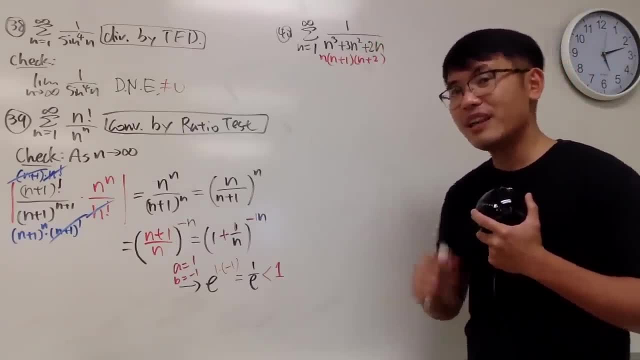 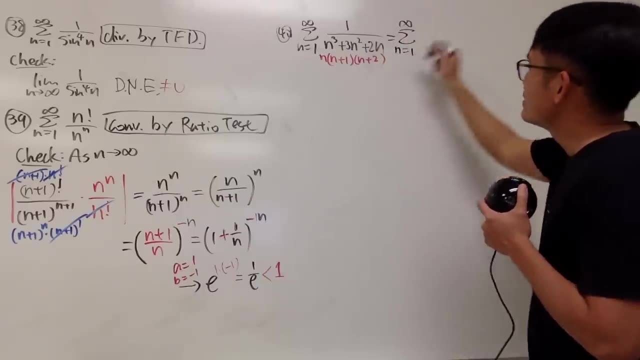 Technically, this right here, it's also going to be a telescoping series. Let me show you, And to do that, we are going to again use partial fractions. Yes, three things on the bottom. It's not that bad at all. 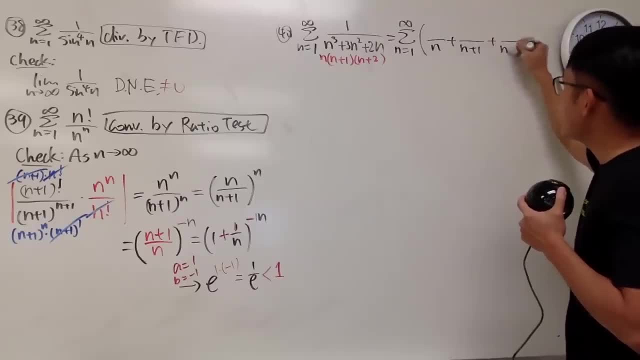 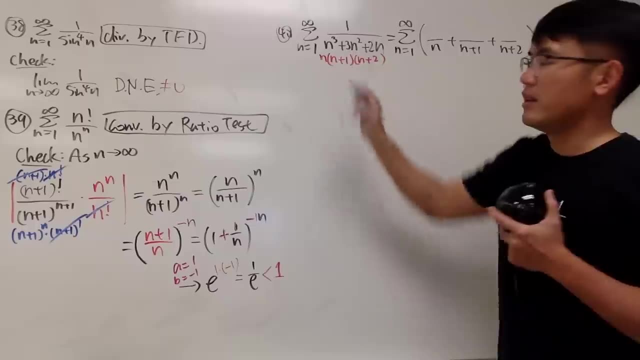 It's the same thing: Cover up, cover up, cover up. All right, So here we go To figure out this number. I will come back here and I will cover up this right here. And how can I make that equal to 0?? 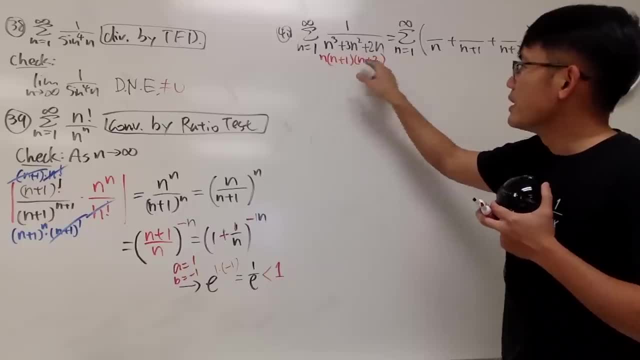 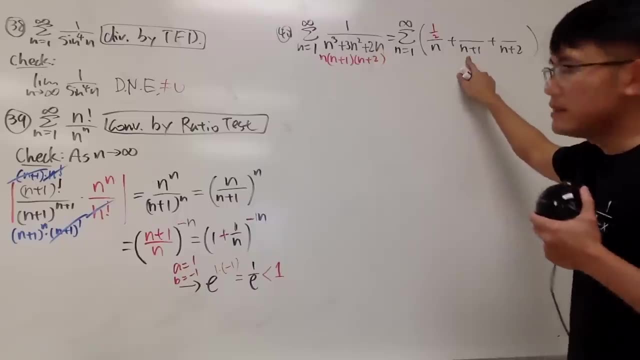 Well, n has to be 0. So 0 here, 0 here. so it's 1 times 2, which is 1 half. Good, Now to make this 0, I will have to. I mean to make this 0, I have to let n equal to negative 1.. 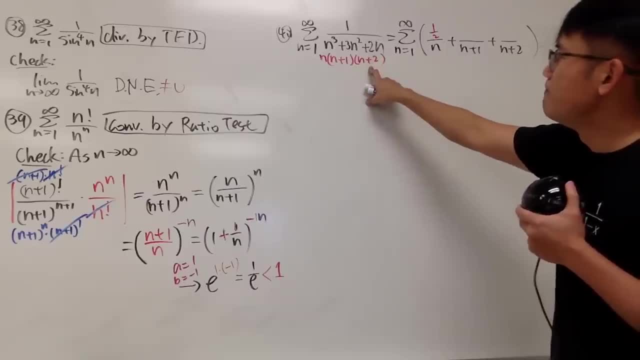 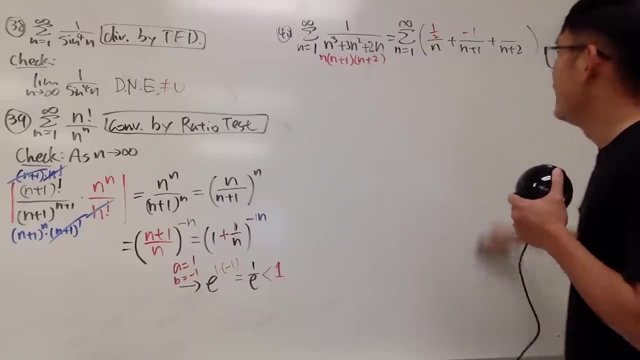 So I have negative 1 times. this is negative 1.. This is 1.. This is negative 1.. So this is negative 1, like that. OK, And then this: right here we have n plus 2.. 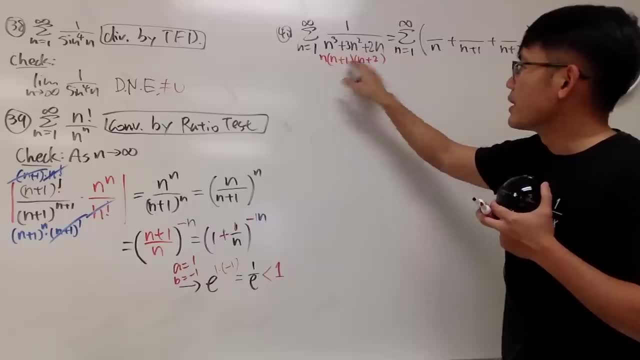 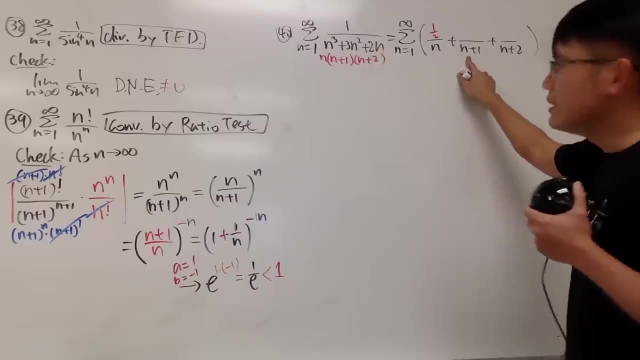 equal to 0?? Well, n has to be 0. So 0 here, 0 here. so it's 1 times 2, which is 1 half Good. Now to make this 0- I mean to to make this 0- I have to let n equal to. 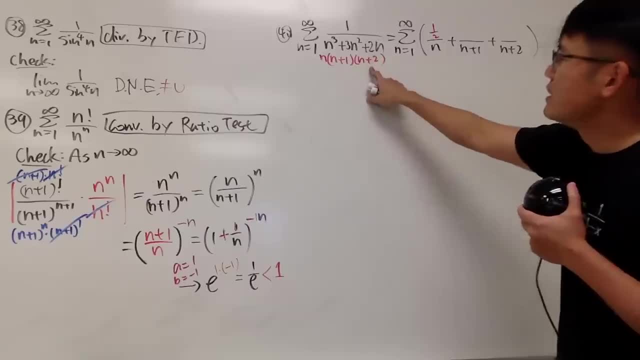 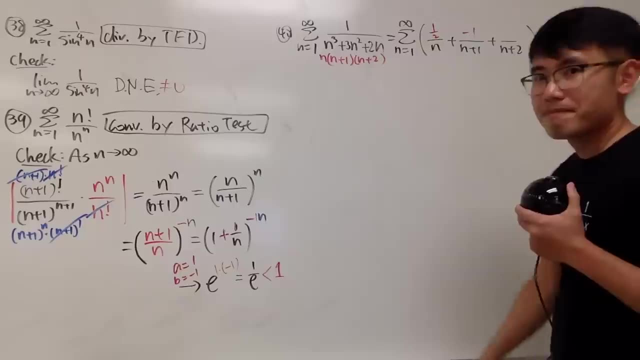 negative 1.. So I have negative 1 times. this is, hmm, negative 1, this is 1, so it's negative 1, so this is negative 1, like that. Okay, And then this: right here we have n plus 2.. Well, I will come back here. 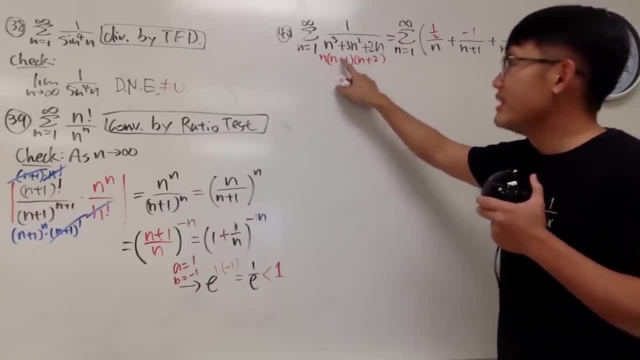 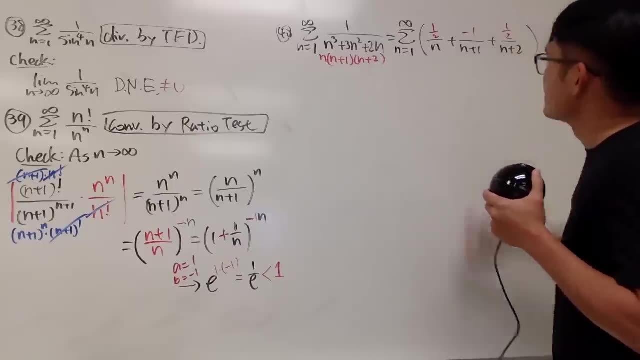 I will plug in negative 2, negative 2- this is negative 2, and this right here is negative. 2 to plus 1 is negative 1. 1 half like that. Okay, so we have all this. I don't know too much about this. 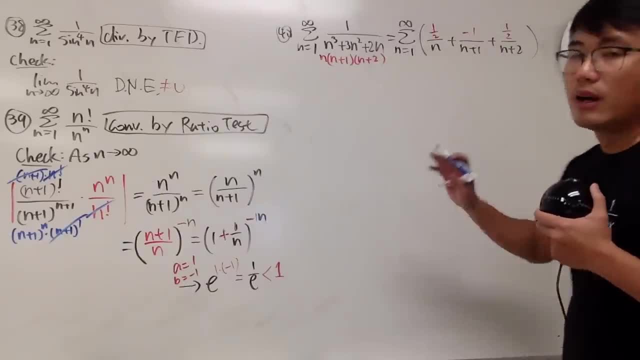 Well, in this case, I will just write down a few terms. and now, here is how we are going to write it down. I will just write down the when n is equal to 1, n is equal to 2 and so on. like this vertically, and we'll. 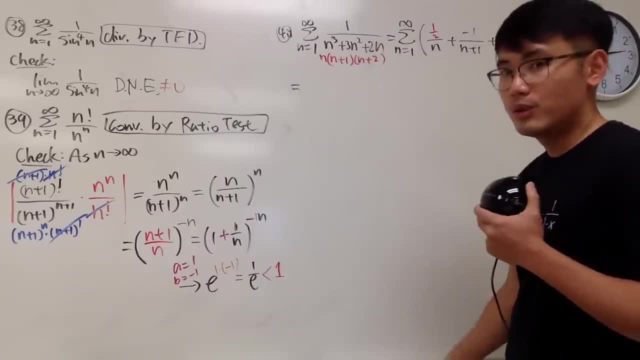 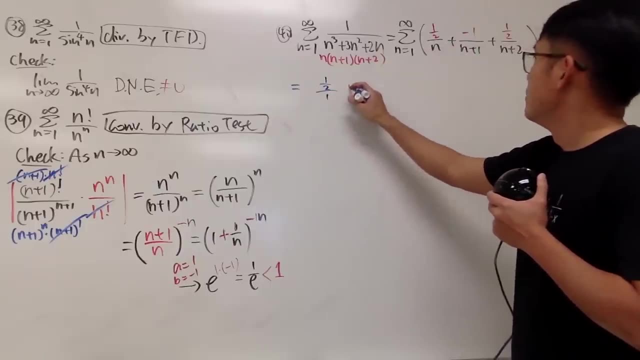 hope to see there might be a pattern that we can do something about it. So when n is equal to 1, we get 1 half over 1 plus negative 1. let me just write it down more neatly so we have more space. plus this right here is 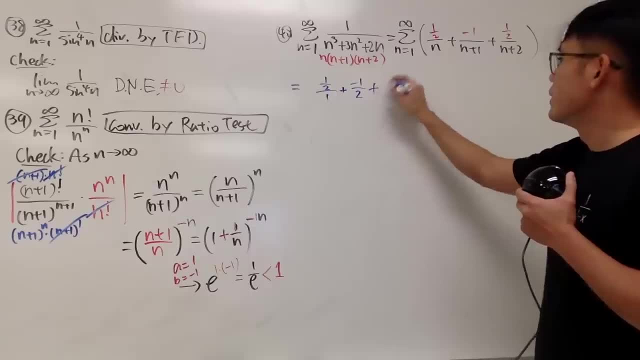 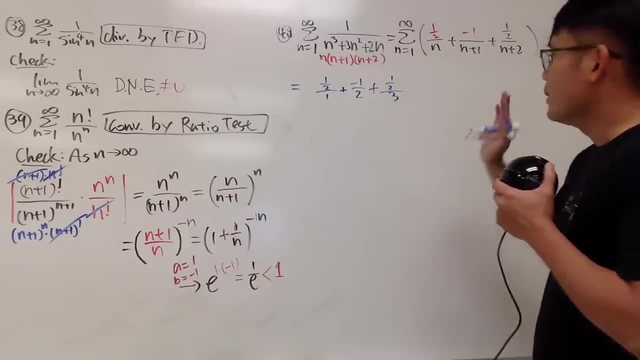 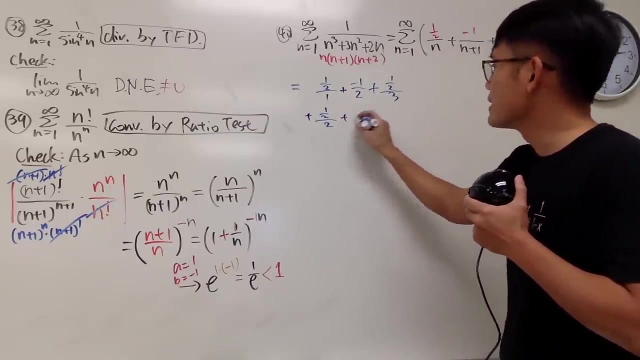 negative 1 over 2, plus 1 half over 3, 1, 2, 3. maybe there is some kind of pattern, Okay, Okay. Next, when n is 2, so we have plus 1 over 2 over 2, plus negative 1. 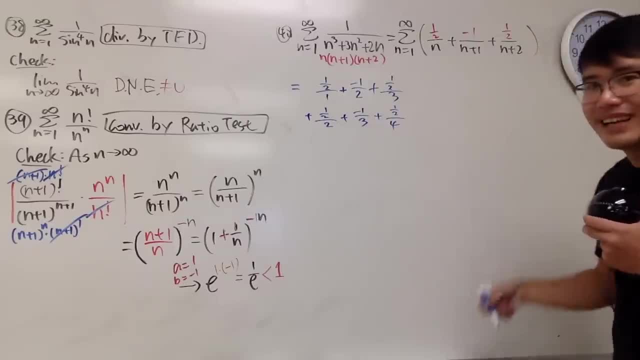 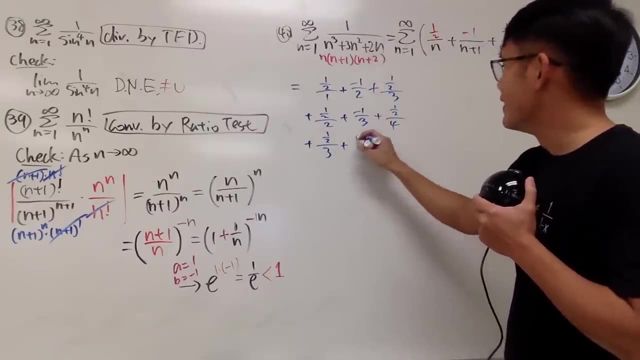 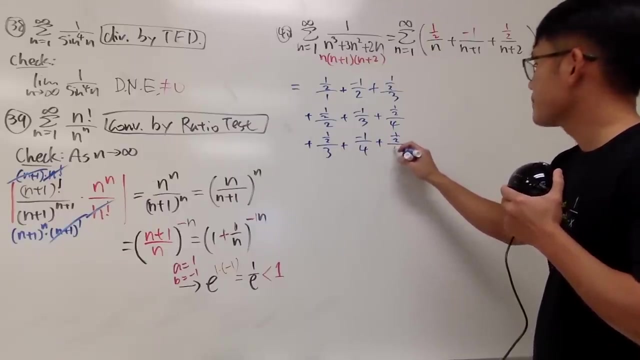 over 3 plus 1 half over 4, right, And then just keep going. let's say 1 half when n is equal to 3. now we have this over 3 plus negative, 1 over 4 plus 1 half over 5. 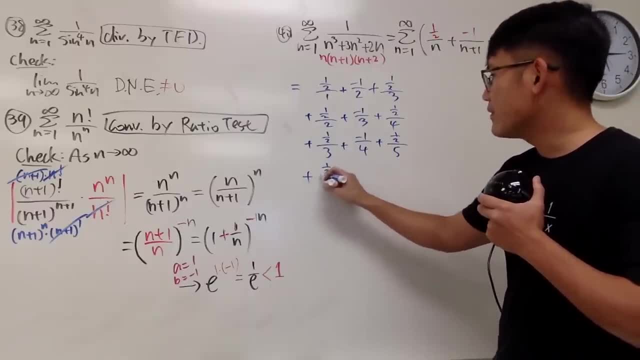 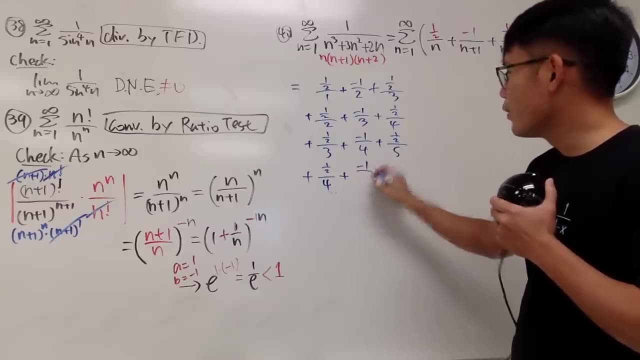 3, 4, 5. good, let's do another one: 1 half over 3, no n is 4. now for this row right n is 4 plus negative, 1 over 5 plus 1 half over 6. 4, 5, 6. 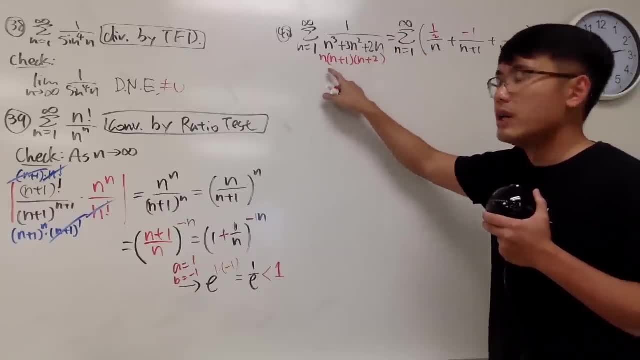 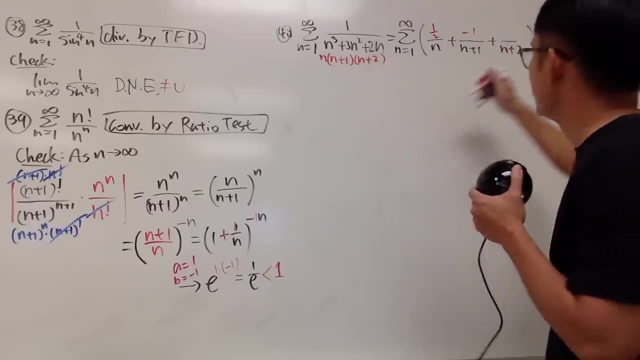 Well, I will come back here. I will plug in negative 2, negative 2.. This is negative 2.. And this right here is negative. 2 to plus 1 is negative 1.. So all in all it's positive 1, half, like that. 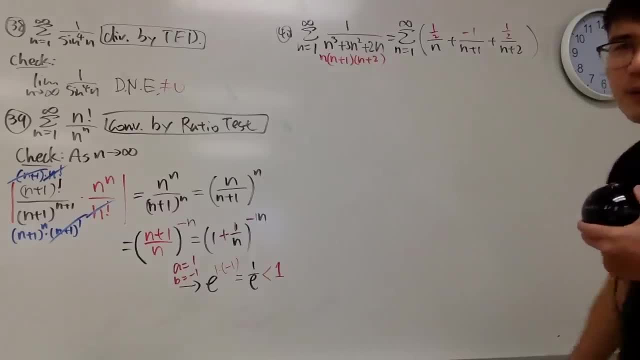 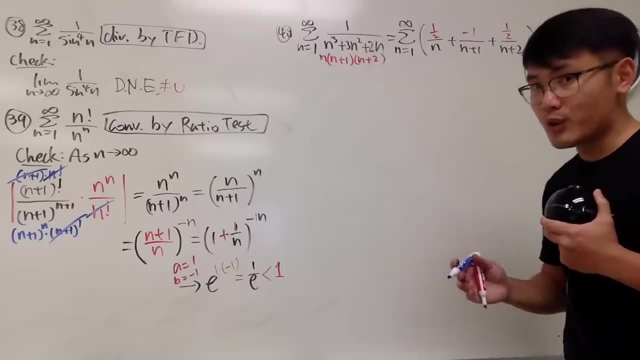 OK, So we have all this. I don't know too much about this. Well, in this case, I will just write down a few terms. And now here is how we are going to write it down. I will just write down when n is equal to 1,, n is equal to 2, and so on, like this vertically. 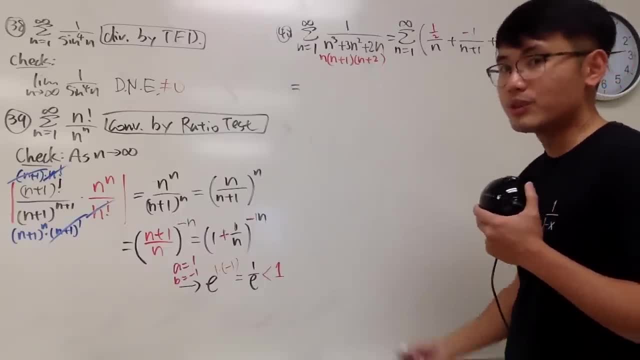 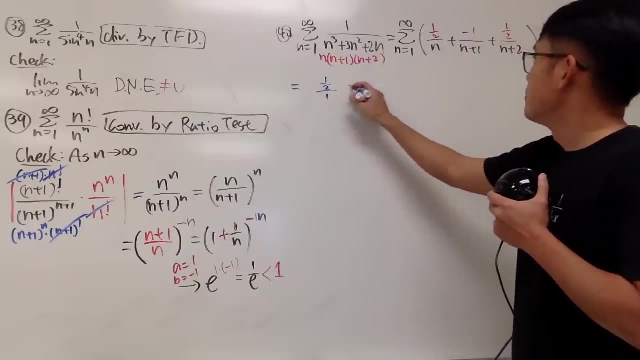 And we'll hope to see there might be a pattern that we can do something about it. So when n is equal to 1, we get 1 half over 1 plus negative 1.. Let me just write it down more neatly so we have more space. 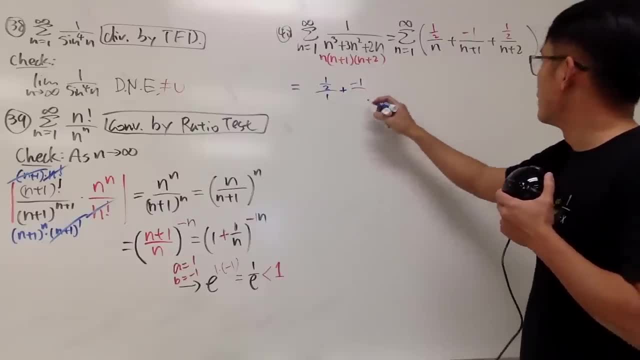 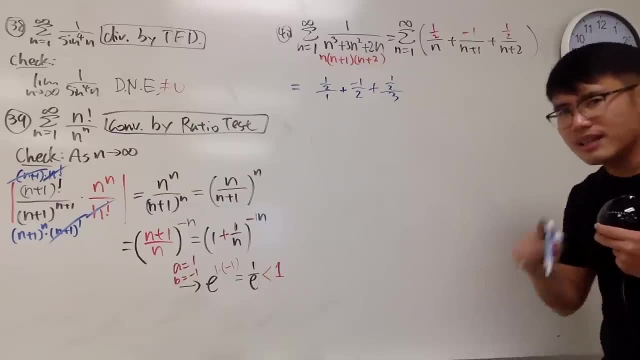 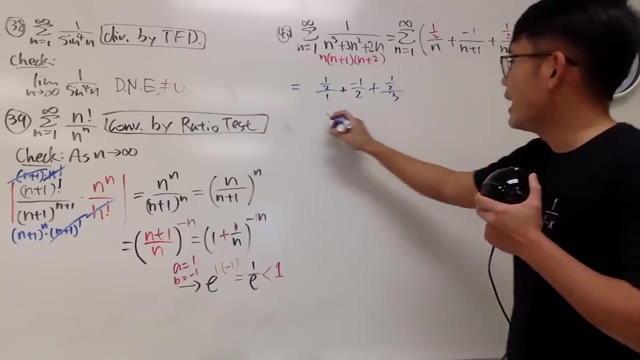 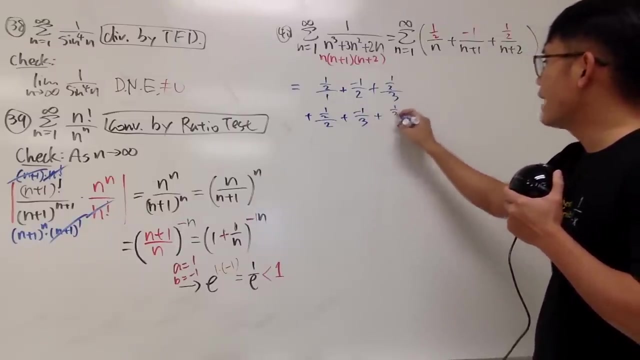 Plus this right here is negative 1 over 2.. Plus 1 half over 3.. 1, 2, 3.. Ah, maybe there's some kind of pattern. OK, OK. Next, when n is 2, so we have plus 1 over 2 over 2, plus negative 1 over 3, plus 1 half over 4.. 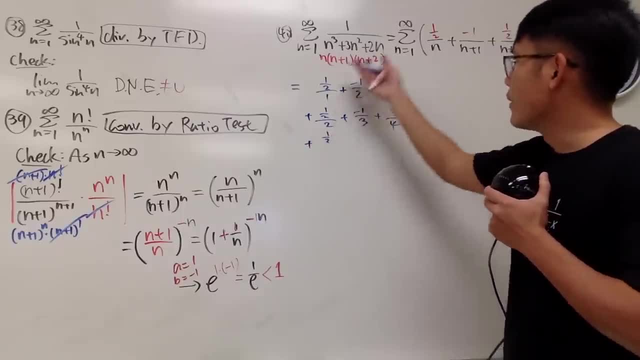 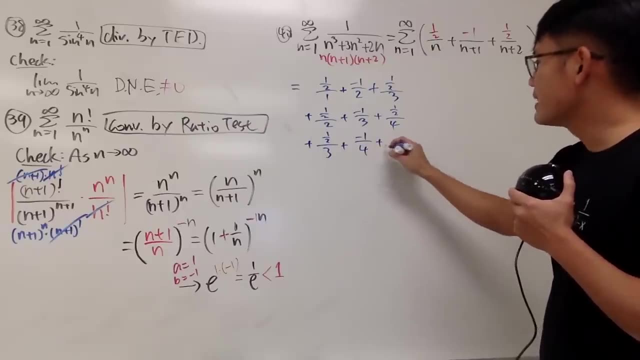 Right, And then just keep going. That's a 1 half When n is equal to 3. now we have this over 3 plus negative 1 over 3.. 4 plus 1 half over 5.. 3,, 4, 5.. 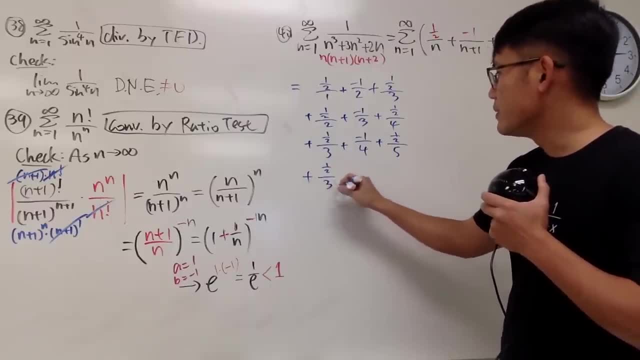 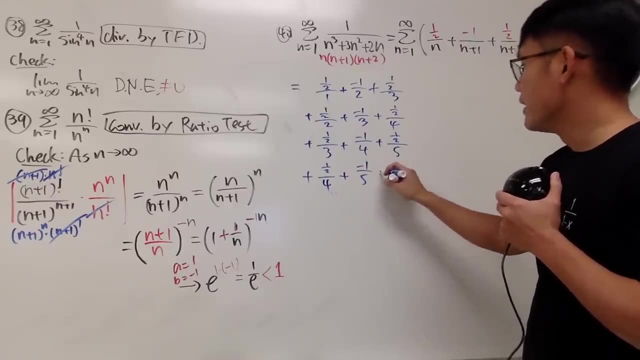 Good, Let's do another one: 1 half over 3.. No n is 4. now for this row, right n is 4 plus negative, 1 over 5 plus 1 half over 6.. 4,, 5, 6.. 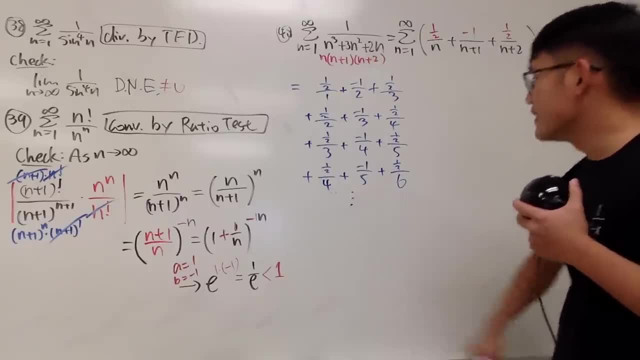 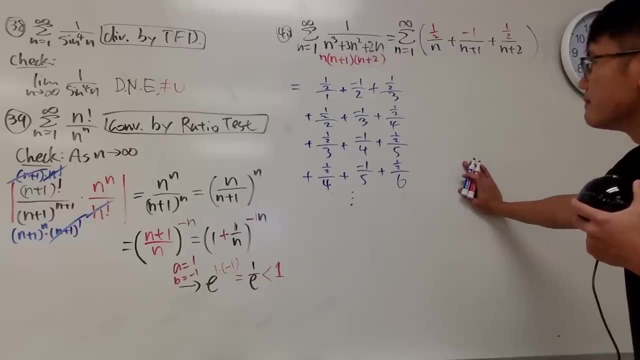 And so on. OK, Of course, dot, dot dot. Hmm, Let's see what in the world we can do with all this Things. Well, check this out. I'm actually going to write this down one more for you guys. 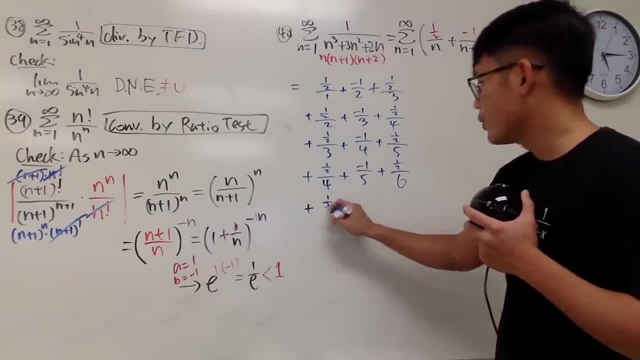 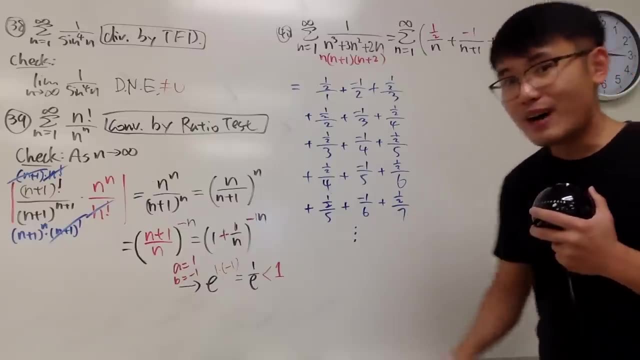 Next one is going to be when n is equal to 5. So we have 1 over 2 over 5, plus negative 1 over 6, plus 1 over 2 over 7.. And then dot dot dot. Now take a look. 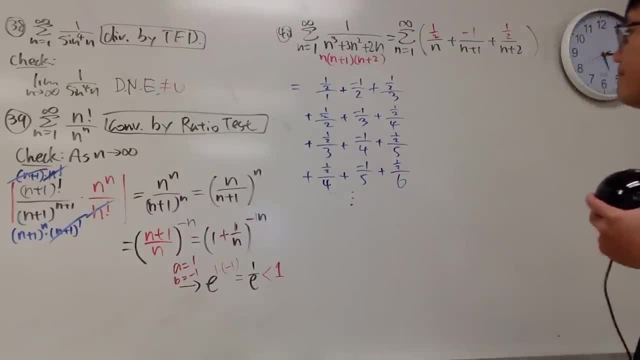 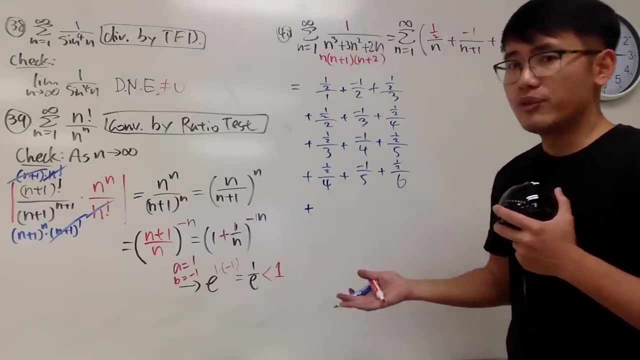 and so on. okay, of course, dot, dot dot. hmm, let's see what in the world we can do with all these things. well, check this out. I'm actually going to write this down one more for you guys. next one is going to be when n is equal to 5. 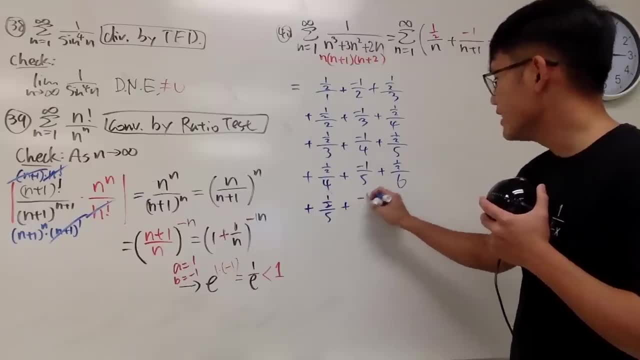 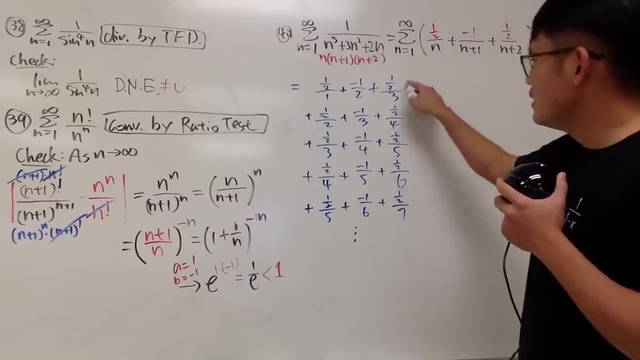 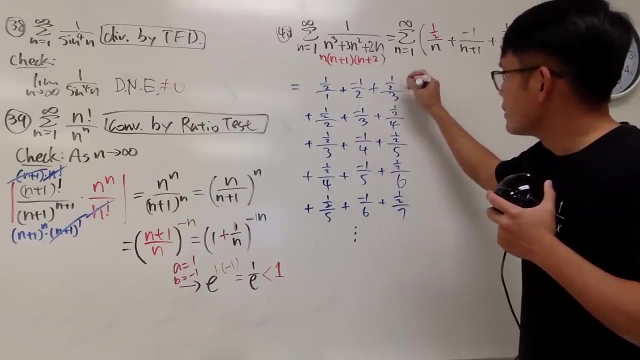 so we have 1 over 2 over 5, plus negative 1 over 6 plus 1 over 2 over 7, and then dot dot dot. now take a look this, this and that: 1 half plus 1 half is 1 minus. 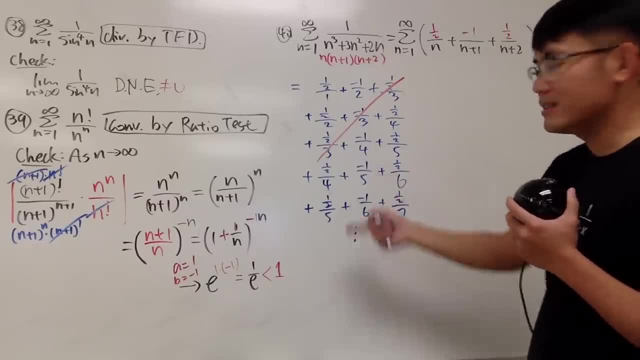 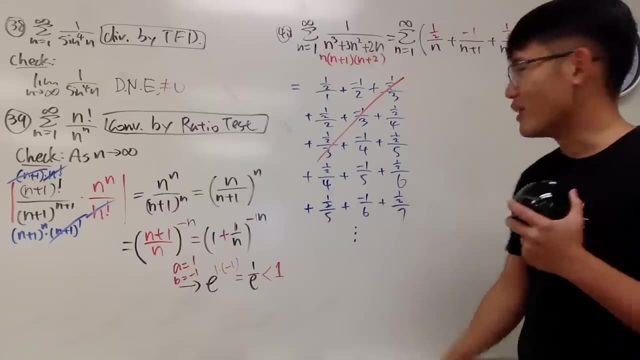 1 is 0, so this guy, I'll just cancel all this guy out diagonally. and is that true? for this? it is denominator being 4, so cancel this out and then cancel this out, and then cancel this out, so on, so on, so on. 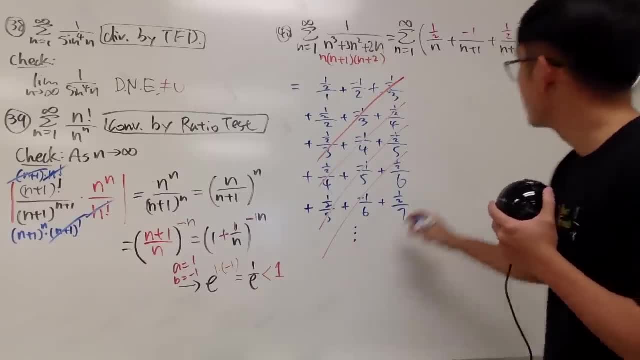 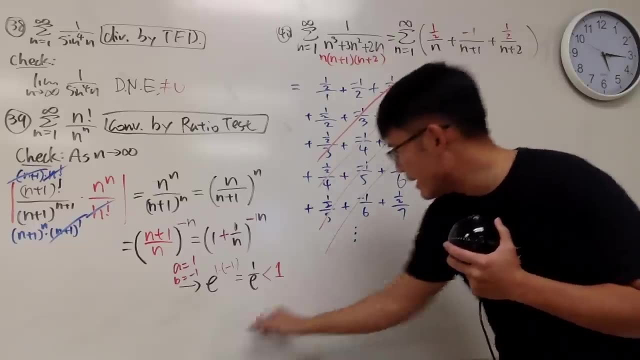 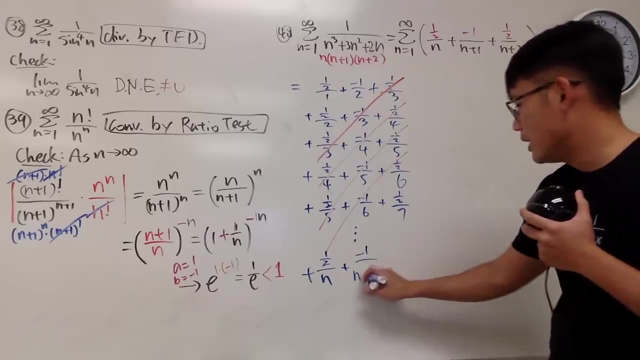 and you know the deal. we should technically write down the nth term right here. so just put down 1 half over n right here, and we are going to get something really cool, right? so, plus negative 1 over n, plus 1, and then, lastly, we have the plus. 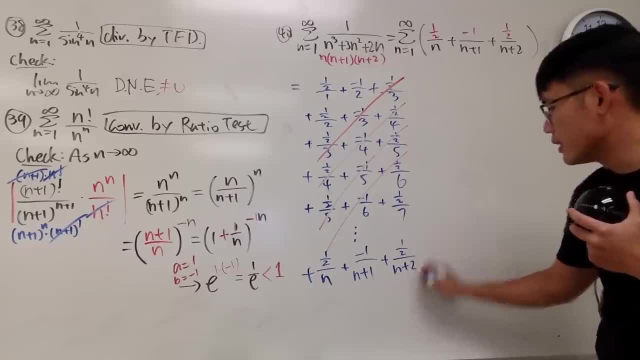 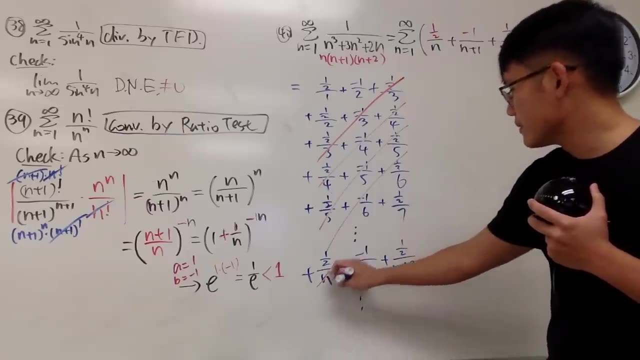 1 half over n plus 1 plus 2, and then, of course again, technically it's still gone forever. so you see that at some point this is going to be gone. and which guy is going to be gone first, if you look at the third row? 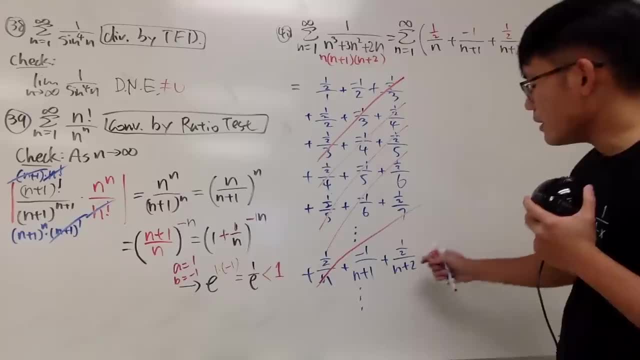 the first guy is going to be gone first, right? so if you just look at this, then you have these two guys right here. but the truth is, it doesn't really matter if you make a small mistake or not, because everybody here is going to 0. 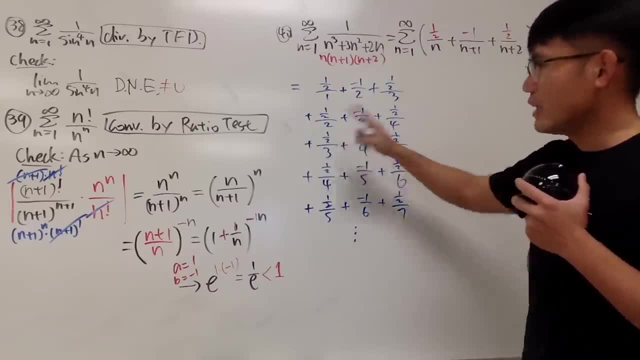 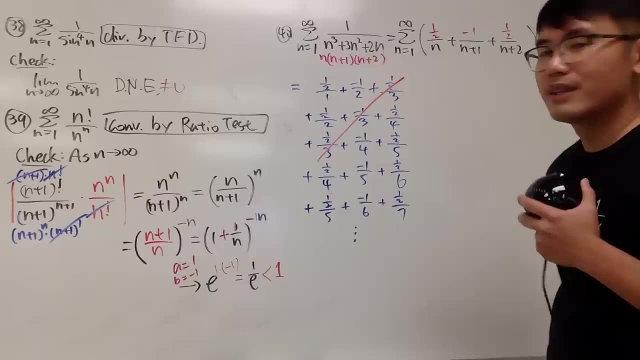 this, this and that 1 half plus 1 half is 1, minus 1 is 0. So this guy, I'll just- how do you say, I'll just- cancel all this guy out Diagonally. 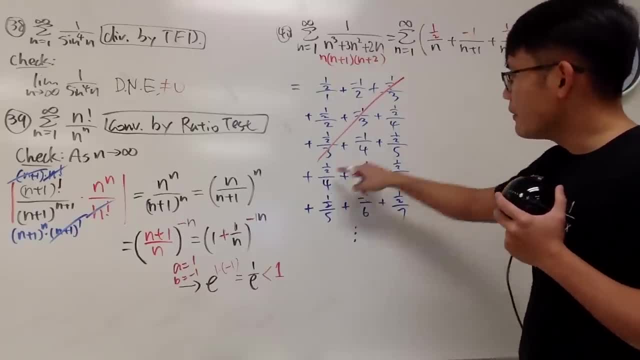 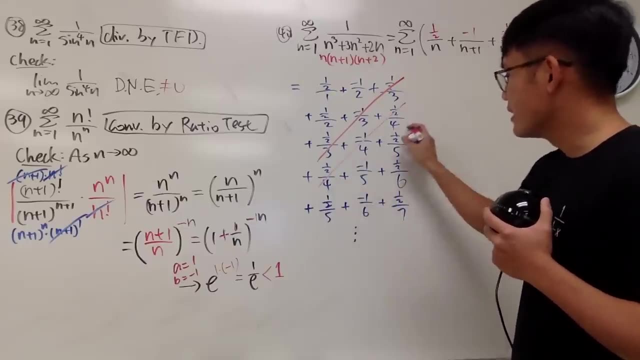 And is that true? for this It is 1 half. 1 half and negative 1. And everybody here have the denominator being 4.. So cancel this out, And then cancel this out, And then cancel this out, So on, so on, so on. 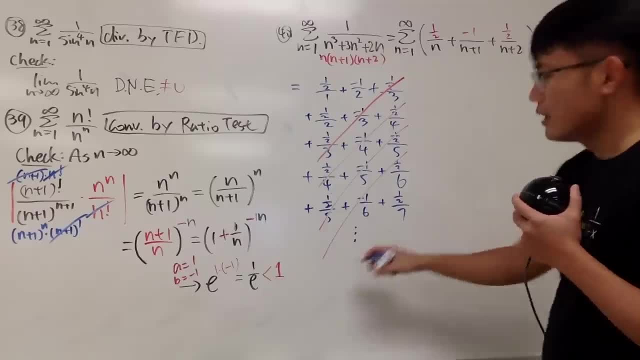 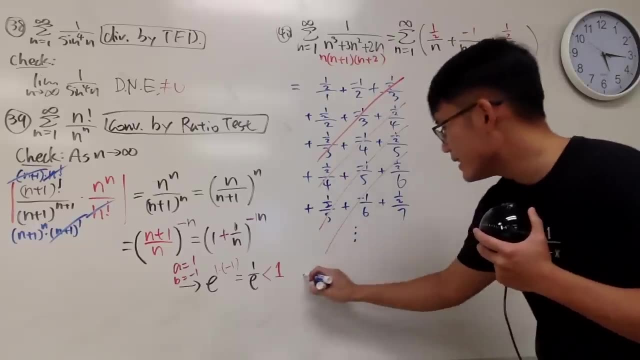 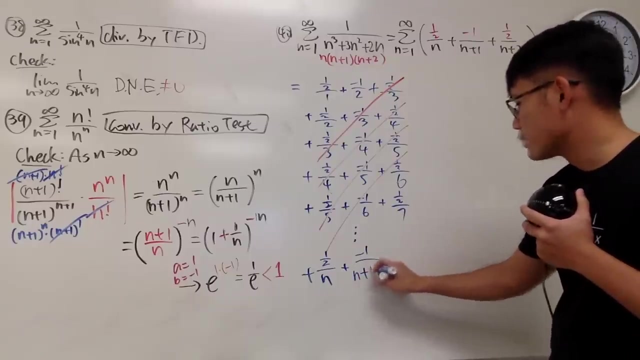 And you know the deal. We should technically write down the nth term right here. So just put down 1 half over n right here And we are going to get something really cool right. So plus negative 1 over n plus 1.. 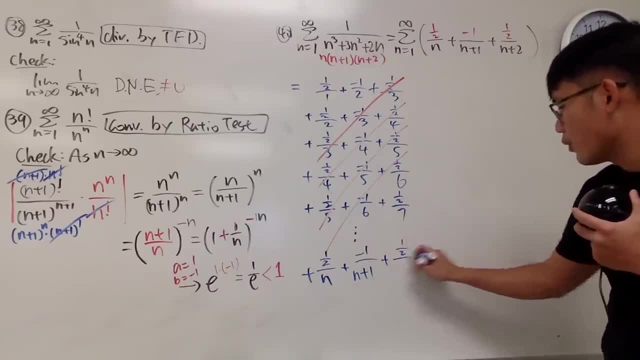 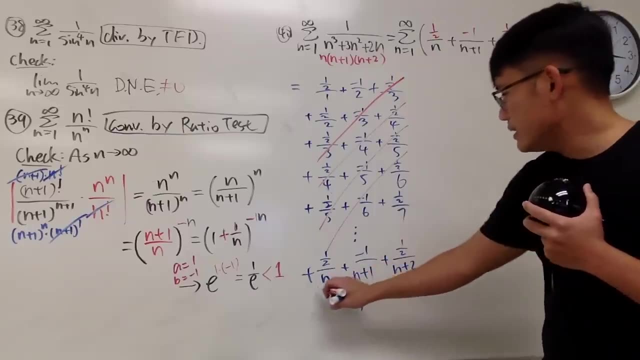 And then, lastly, we have the plus 1, half over n plus 2.. And then, of course, again, technically it's still gone forever. So you see that at some point this is going to be gone, And 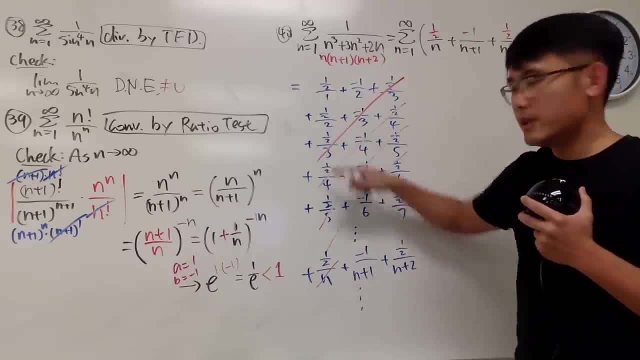 which guy is going to be gone first. If you look at the third row, the first guy is going to be gone first, right? So if you just look at this, then you have these two guys right here. But the truth is. 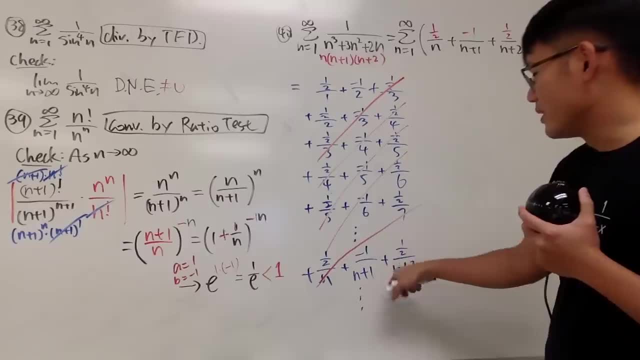 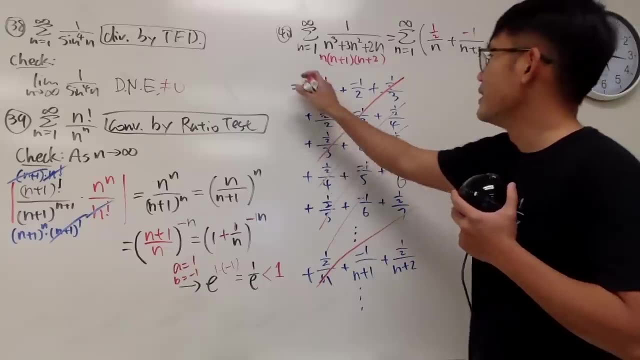 it doesn't really matter if you make a small mistake or not, because everybody here is going to 0.. So anyway, here's the deal. I hope I can add fractions right, because it's kind of tiring, But you still take the. 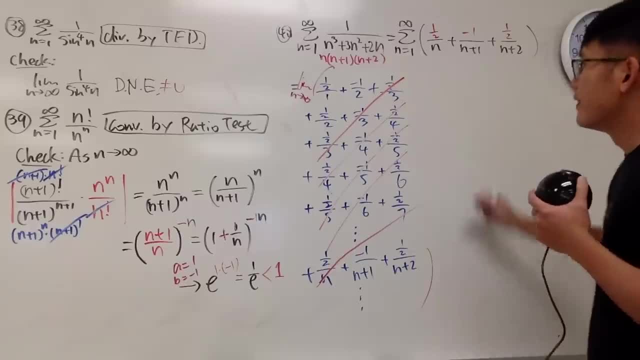 limit as n goes to infinity of all this expression. Now our surviving terms are: this is just 1 half. and then we have the minus 1 half. Oh god, that's 0. So nice. And then here we have. 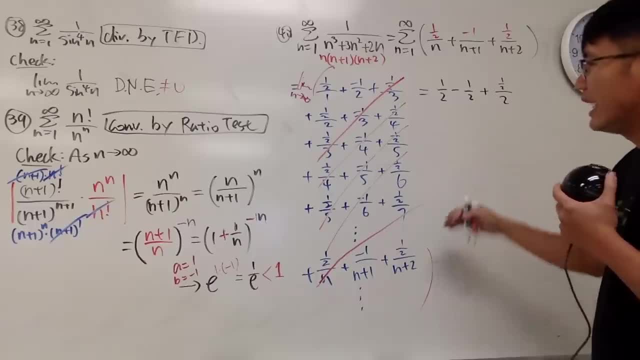 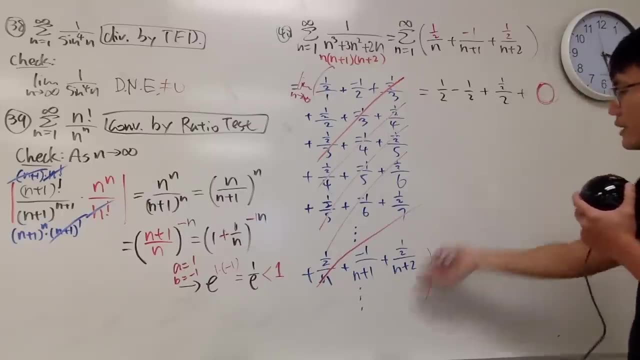 plus 1 over 2 over 2, and here you just have a bunch of 0s And then plus 0s, and we'll just put on 0s right here. right, Because this guy goes to 0,, this guy. 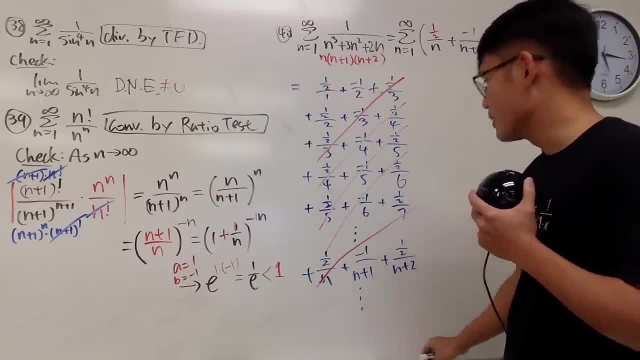 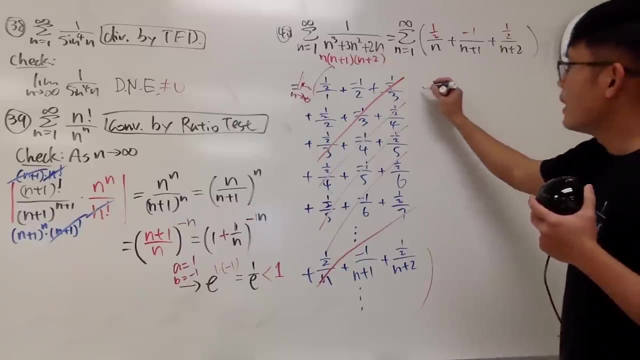 so anyway, here's the deal. I hope I can add fractions, right, it's not tiring, but you still take the limit as n goes to infinity of all this expression. now our surviving terms are: this is just 1 half, and then we have the minus 1 half. 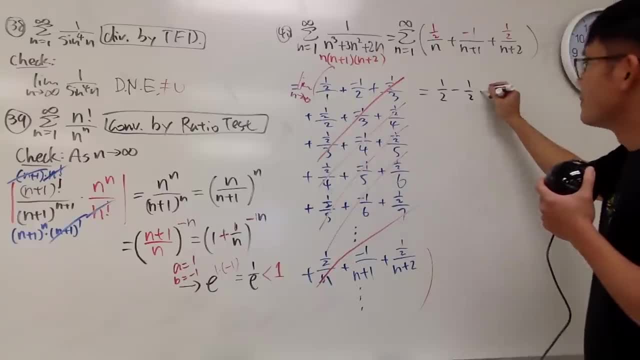 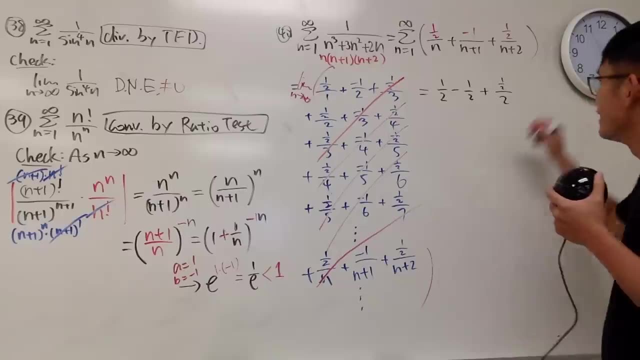 oh god, that's 0, so nice. and then here we have plus 1 over 2, over 2, and here you just have a bunch of 0s and then plus 0s, and I'll just put on 0s right here, right, because? 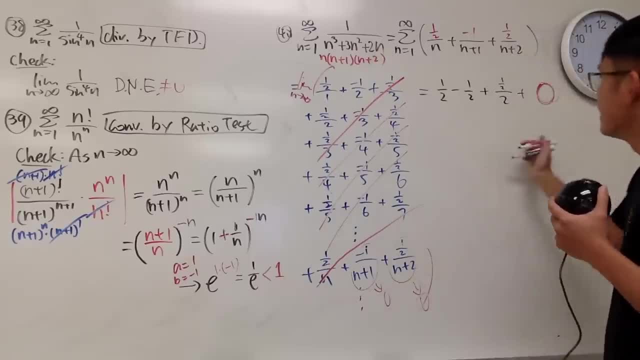 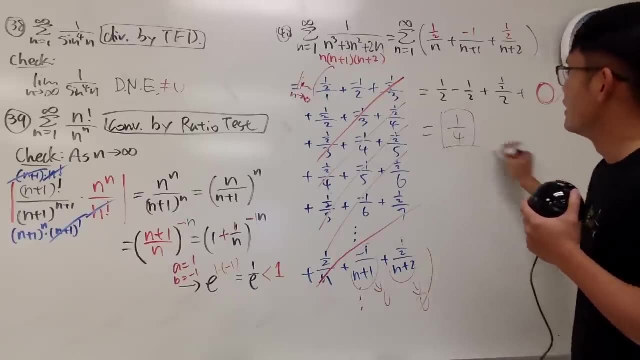 this guy goes to 0, this guy also goes to 0. so, all in all, the answer is 1 over 2 over 2, which is 1 over 4. whew converges to 1 over 4. yes, yes, very, very cool, very, very cool. 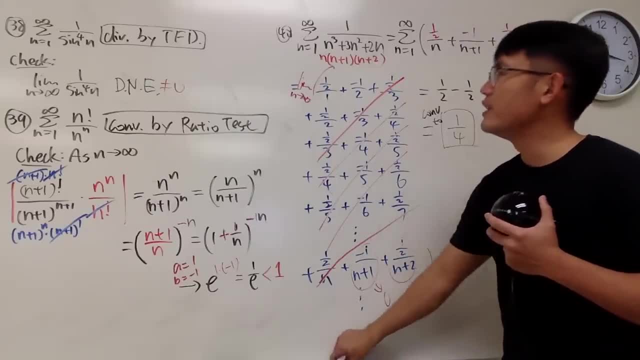 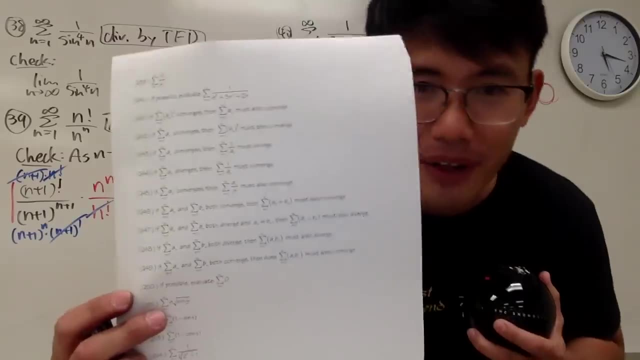 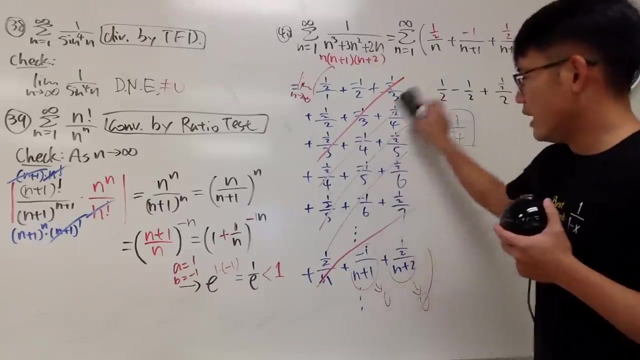 right. so this is very, very nice. that's 40 questions. now here is some special thing for you guys right here. this is more of the true false question and depends on your teacher. sometimes I may just ask like true, false questions and you will have to provide. 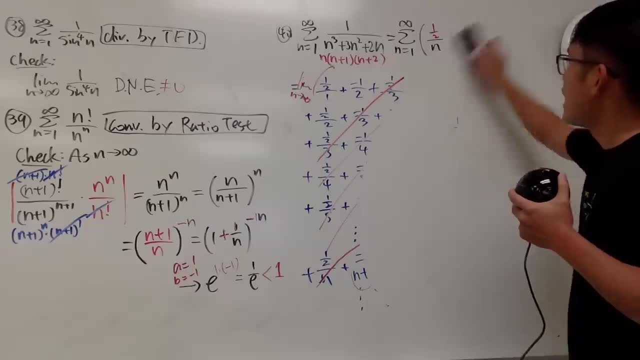 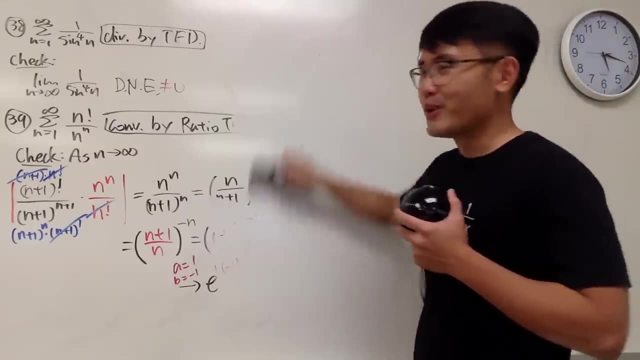 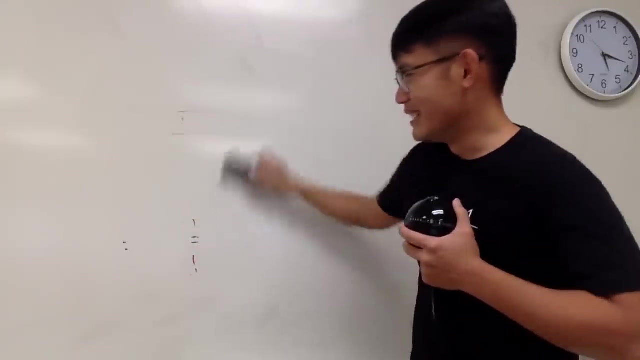 some quick reason, or maybe counter examples, why the statement is true or false. and sometimes you can also put this into multiple choice and then say which of the following is true and which of the following is false, and you can put like 5 statements and I don't know which one. 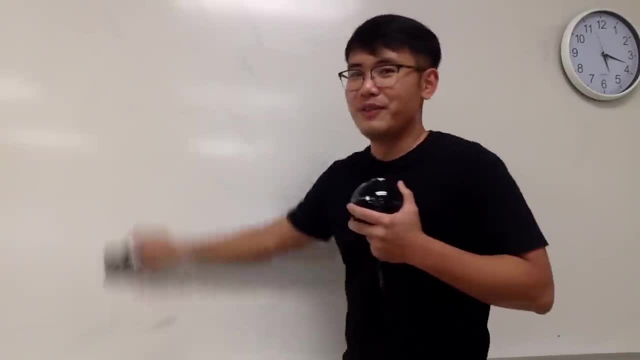 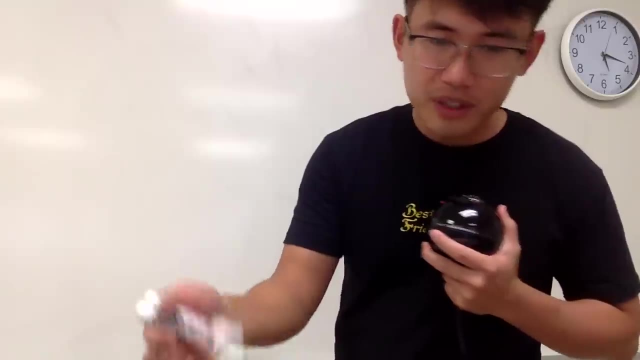 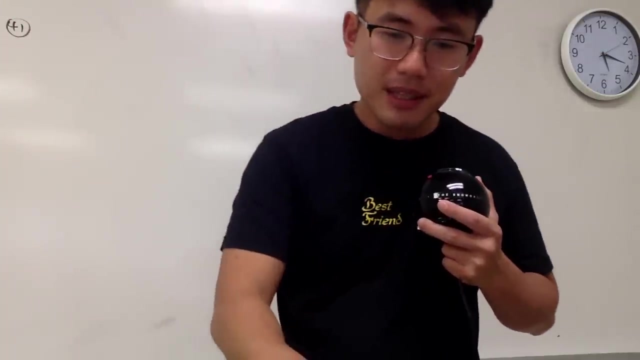 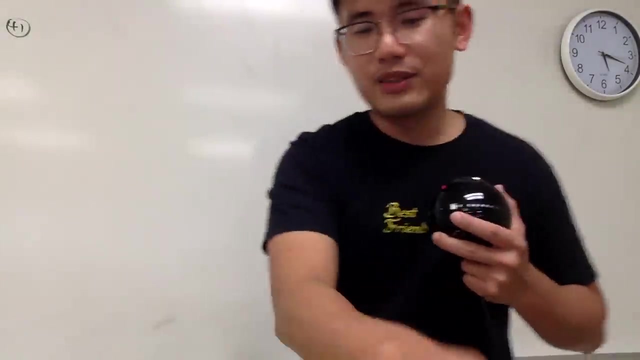 the students will like or hate more, but it depends on how I feel. when I read the exams, I guess: okay, so here we go, number 41 right here, and I'm not going to write down the statement. okay, so if a n square converges then, oh, I think I still have to write down. 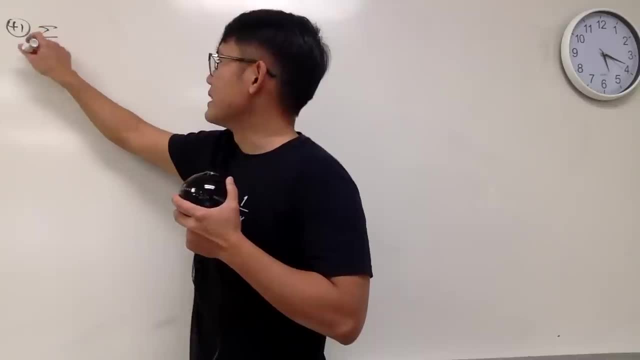 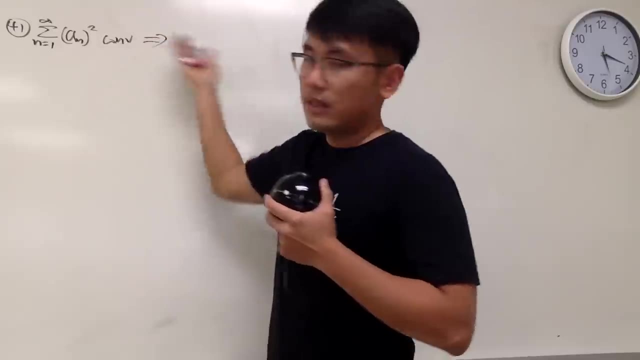 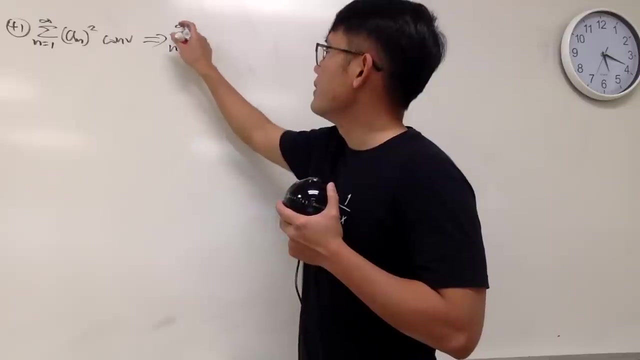 the statement. so I will just put this down in like the simplest way: if n goes from 1 to infinity, sum a n. if this right here converges, then the error means implies: then this implies that the series as n goes from 1 to infinity of a n. 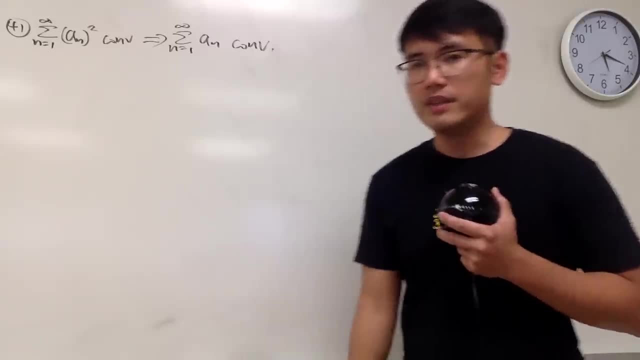 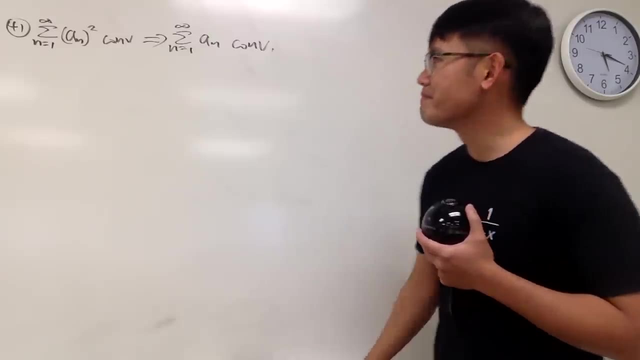 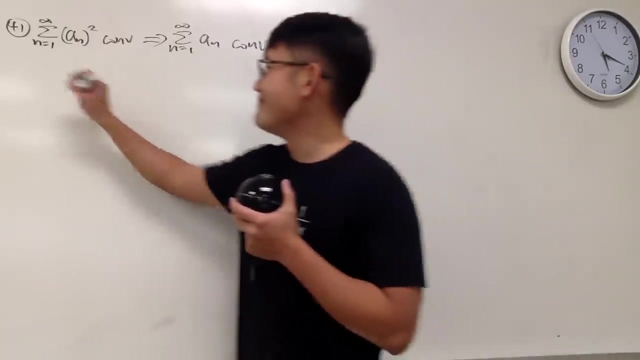 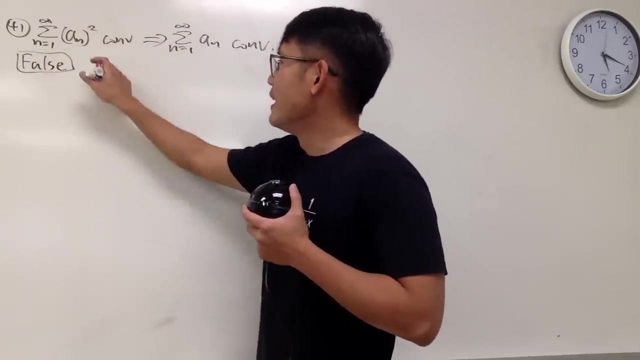 must also converges, true or false? if it's true, just give, just give a quick reason. if it's false, you have to provide counter example. false right, and I'll just, you know, do this real quick for you guys. counter example right a n. you can take 1 over n for this. 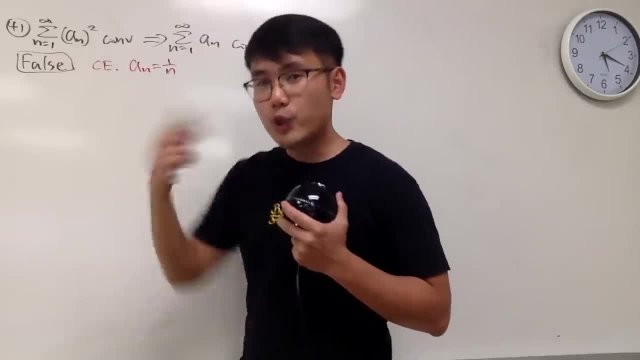 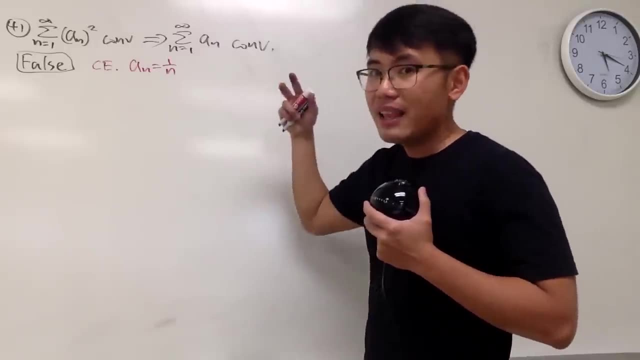 and, as you can see, if you put 1 over n in here, you square that first. you get 1 over n square in the sum. that converges. that's true, but if you put 1 over here, that diverges. so this right here will be a counter example. 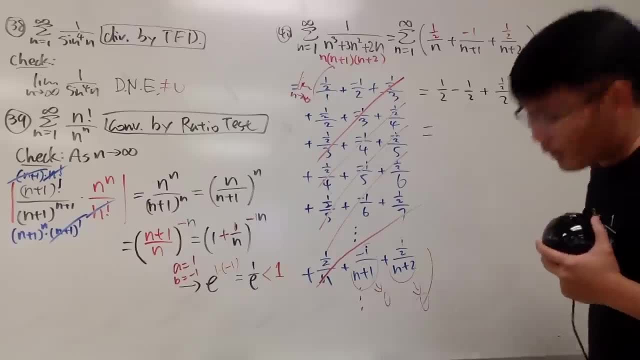 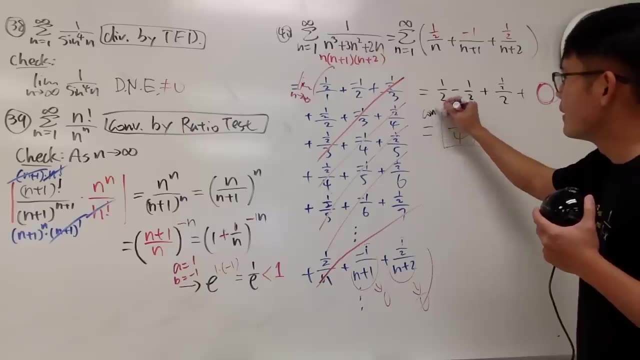 also goes to 0. So, all in all, the answer is 1 over 2 over 2, which is 1 over 4.. Woo Converges to 1 over 4.. Yes, Yes, Very, very cool, Very, very cool right. 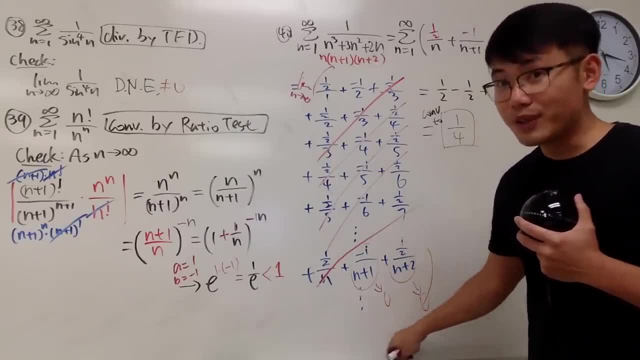 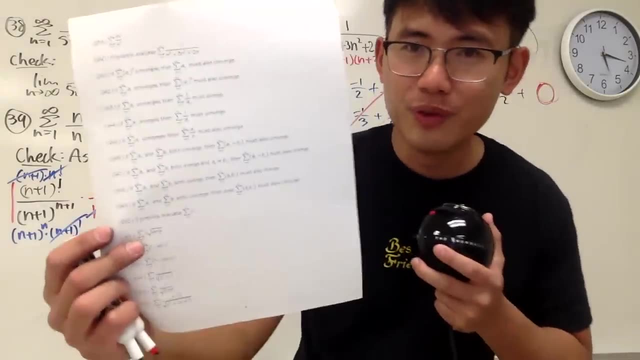 So this is very, very nice. That's 40 questions. Now here is some special thing for you guys right here. This is more of the true-false question and depends on your teacher. Sometimes I may just ask like true-false questions. 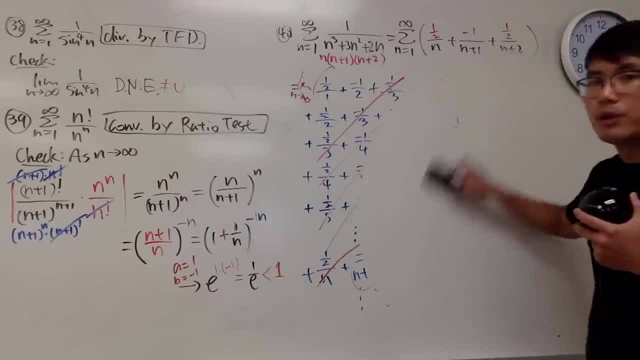 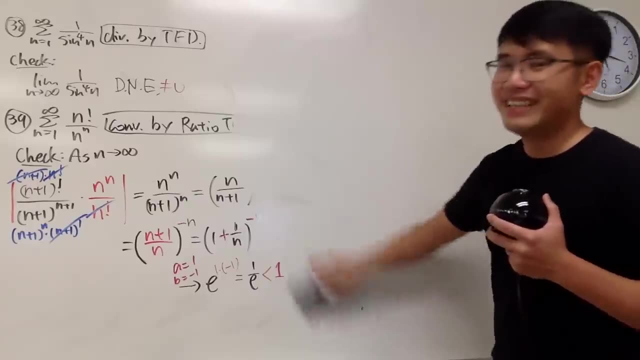 and you will have to provide some quick reason, or maybe counter-examples, why the statement is true or false. And sometimes you can also put this into multiple choice and then say which of the following is true and which of the following is false. 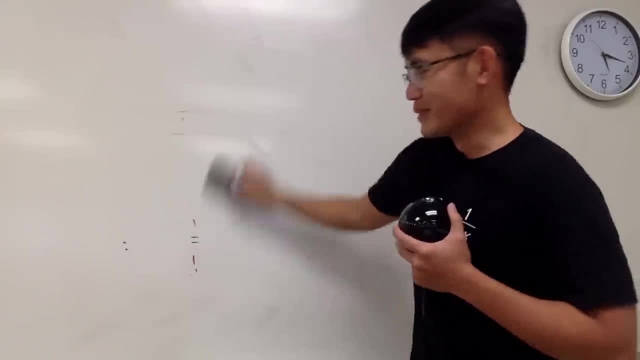 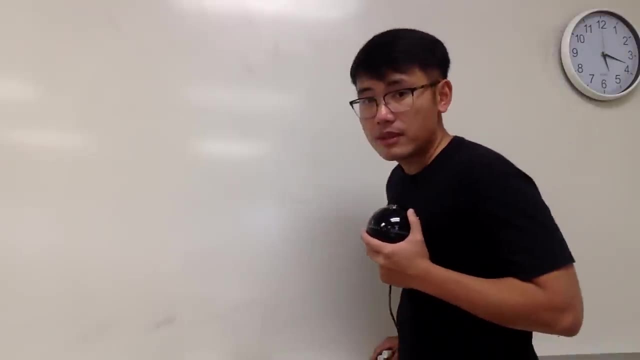 And you can put like 5 statements And I don't know which one the students will like will hate more. but it depends on how I feel when I write the exams. I guess Okay, So here we go. Number 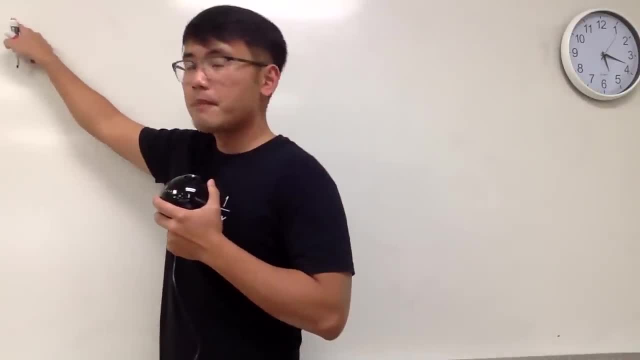 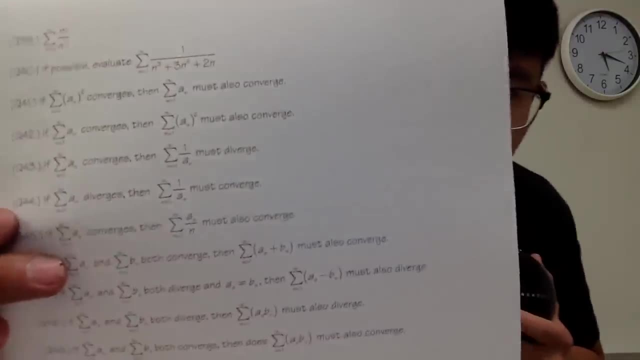 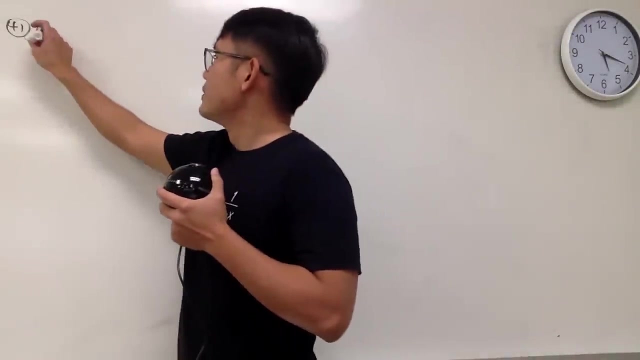 41, right here, And I'm not going to write down the statement. okay, So if AN squared converges, then- oh, I think I still have to write down the statement, So I'll just put this down in the like. 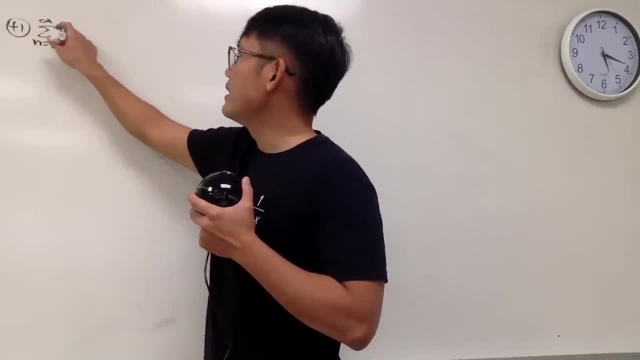 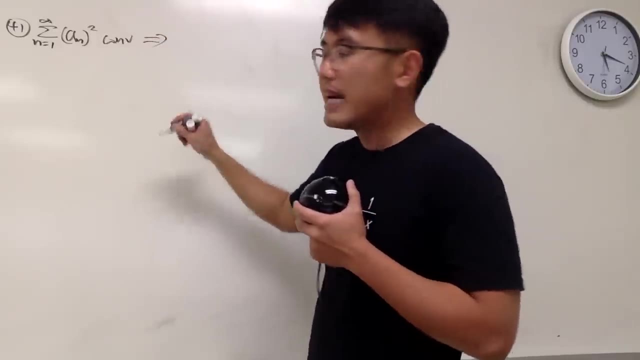 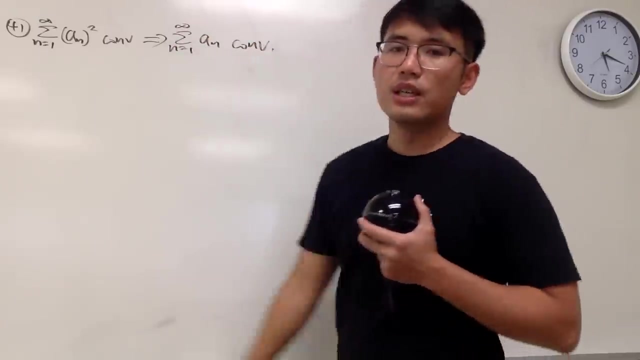 the simplest way: If N goes from 1 to infinity, some AN, if this right here converges, uh, the error means implies then in- this implies that the series, as N goes from 1 to infinity of AN must also converges, true or false? 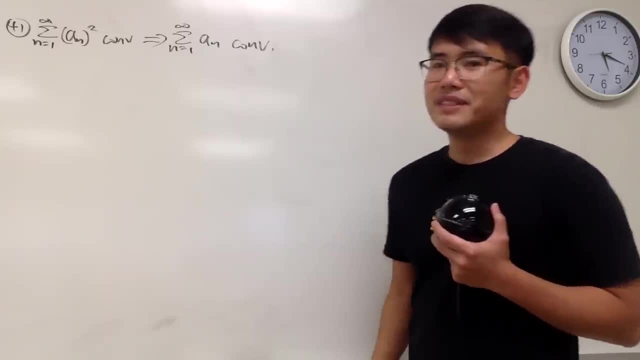 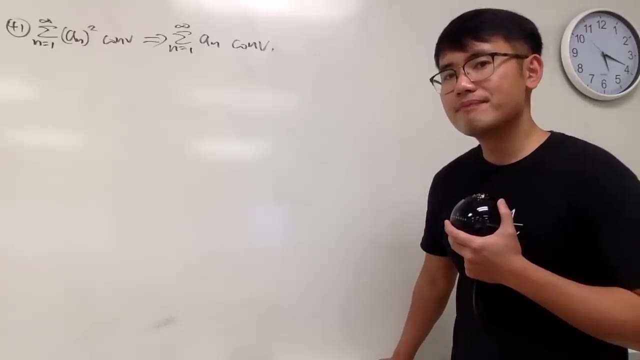 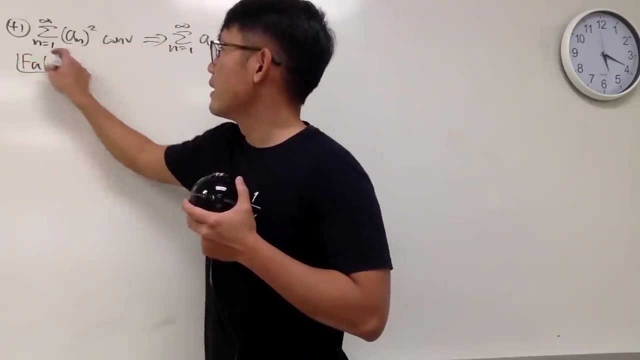 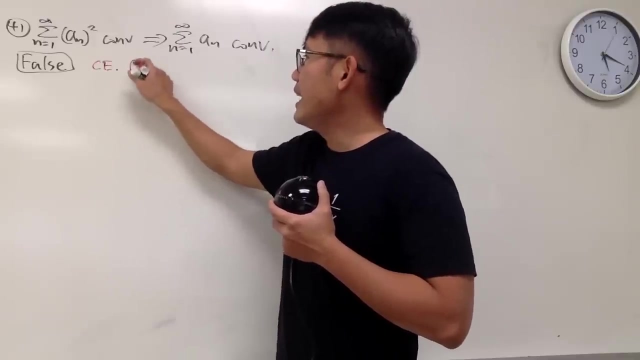 If it's true, just give a quick- just give a quick reason reason. If it's false, you have to provide counter-example False. And I'll just do this real quick for you guys. Counter-example a- n. you can take 1 over n for this And as 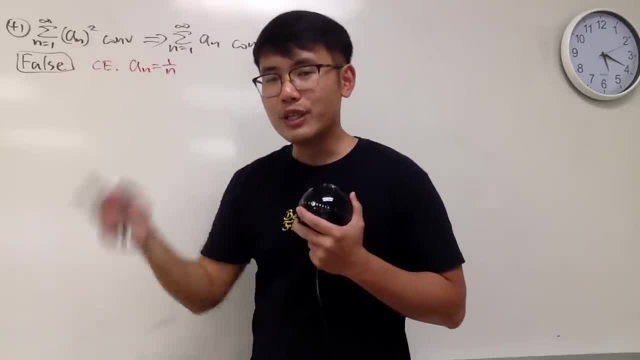 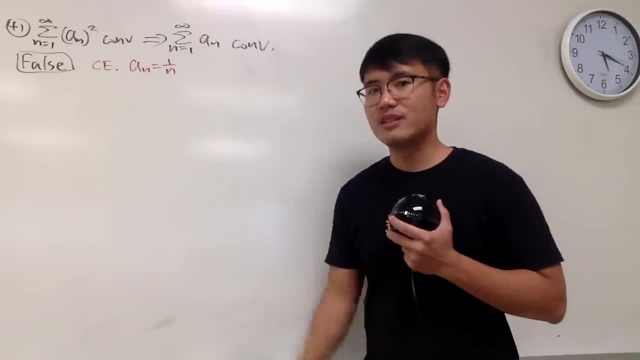 you can see, if you put 1 over n here you square that first. you get 1 over n squared In the sum that converges. That's true, But if you put 1 over here, that diverges. So 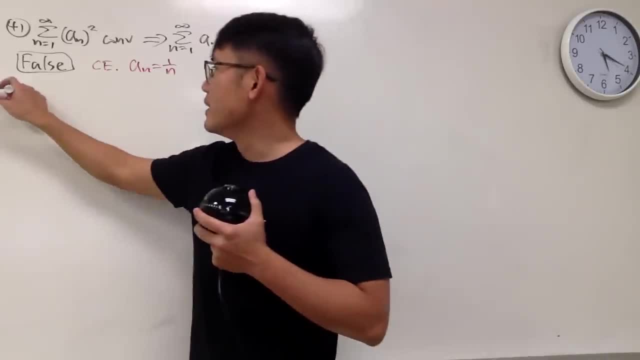 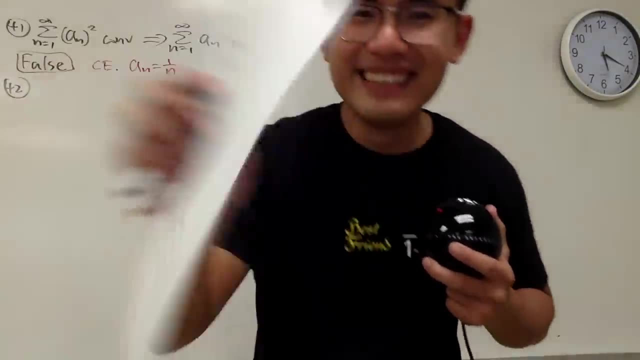 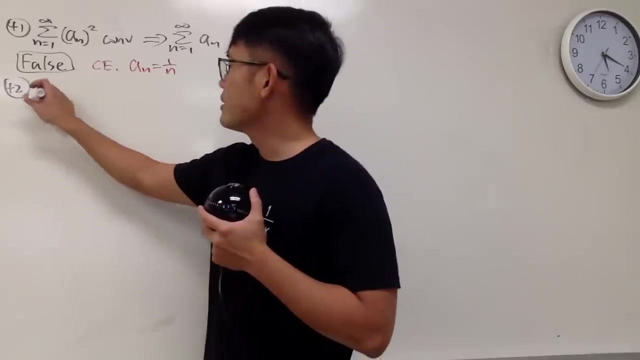 this right here will be a counter-example, So I think I'll just go over it like this, without putting down too much, So that way we can speed up the process right here. OK, The other way, if we have this being converged the other way, does it converge The sum as? 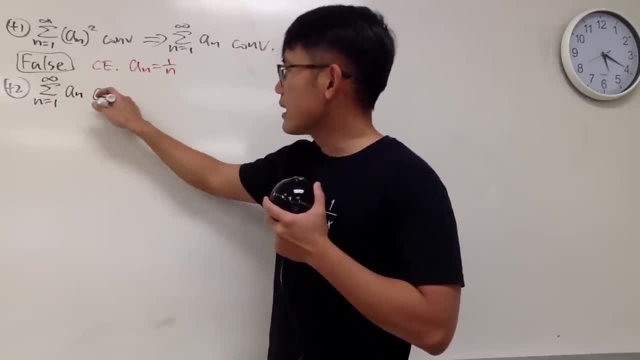 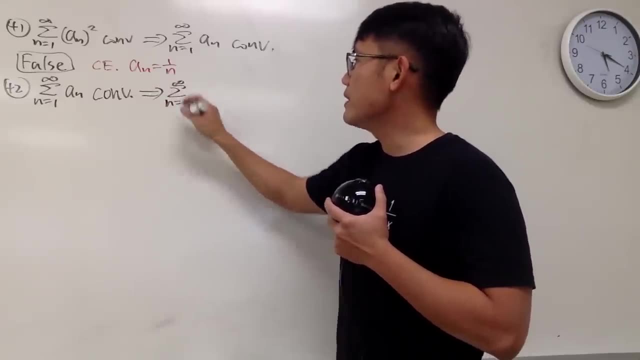 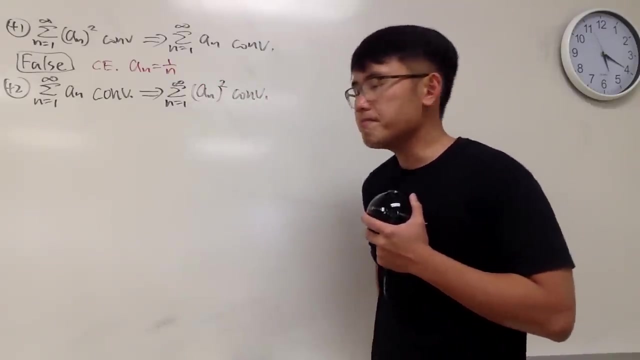 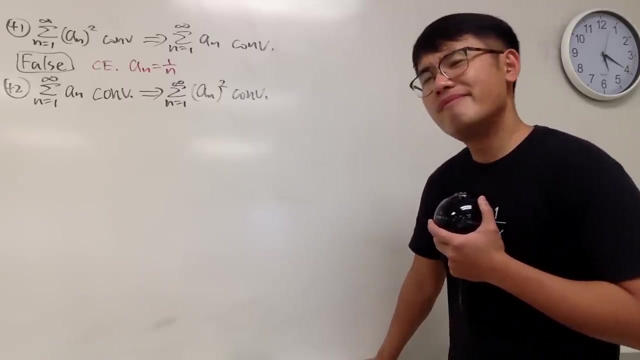 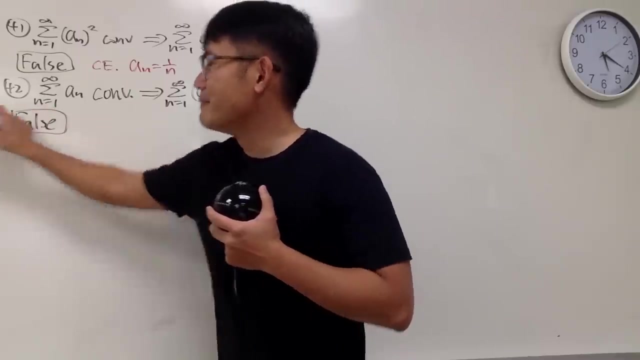 n goes from 1 to infinity. If this converges, do we must have the square version, namely the sum, as n goes from 1 to infinity, of a n squared also converge. Hmm, Let's see, Still false. Give me a counter-example. 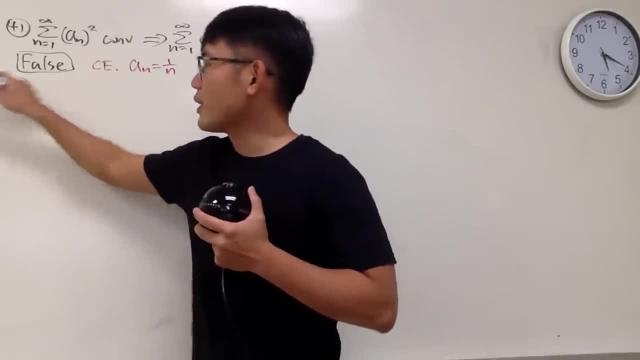 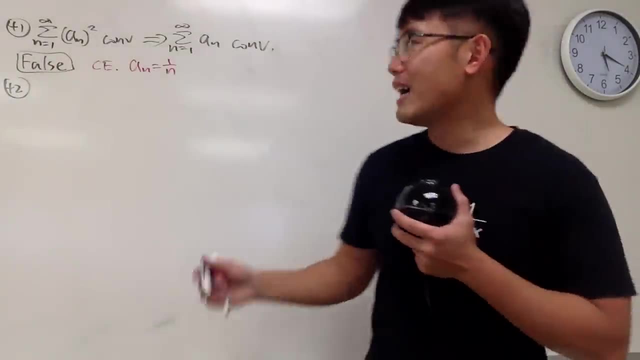 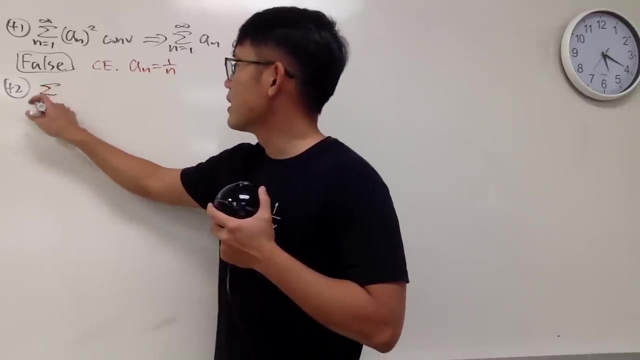 all right, so I think I'll just go over it like this, without putting down too much, so that way we can speed up the process right here. okay, the other way, if we have this being converged the other way, does it converge the sum as n goes from 1 to infinity? 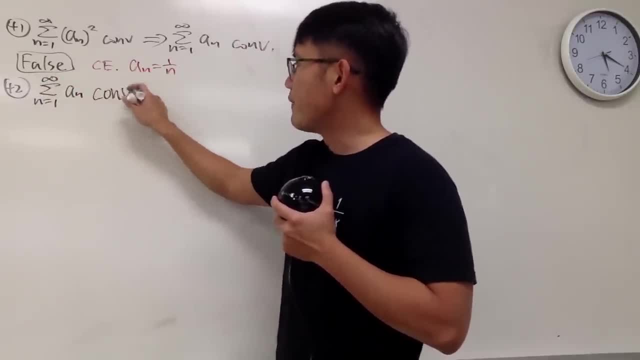 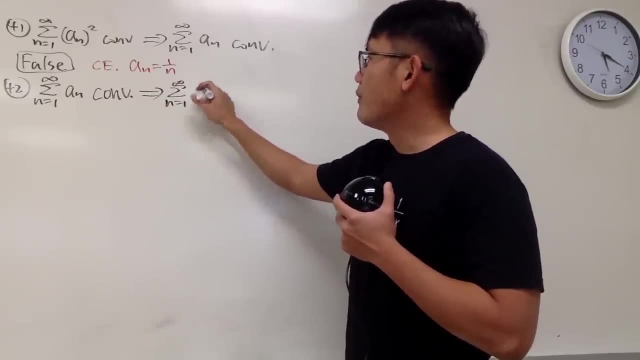 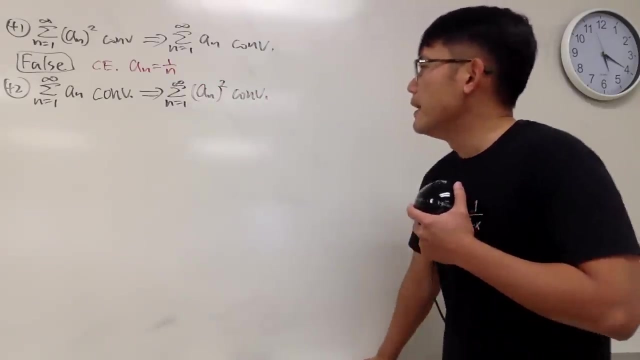 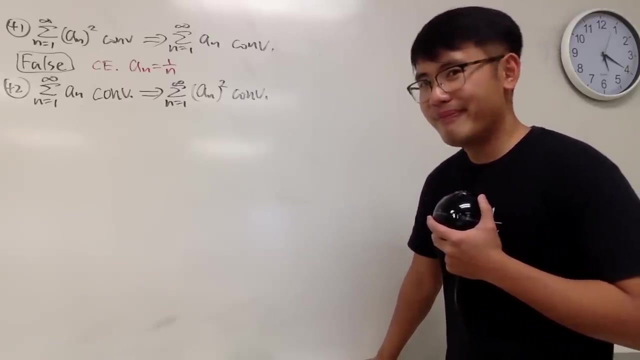 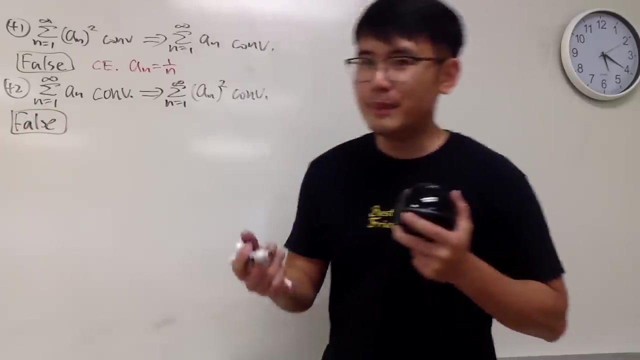 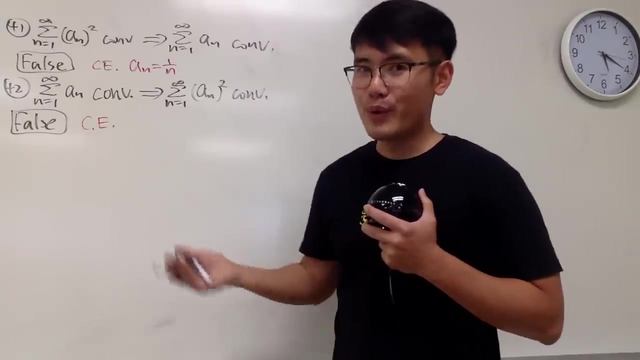 if this converges, do we must have the square version, namely the sum, as n goes from 1 to infinity, of a n square also converge? hmm, let's see, still false. give me a counter example. okay, I'll tell you counter example right here. I will just show you. 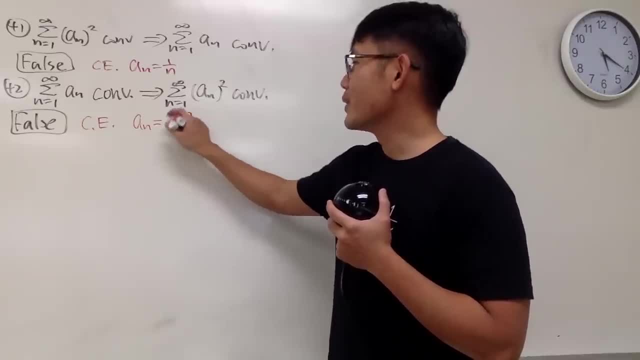 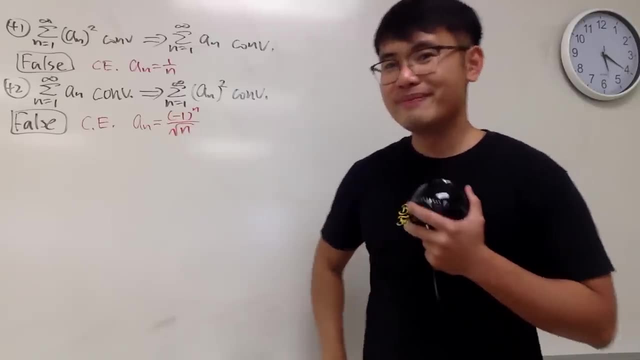 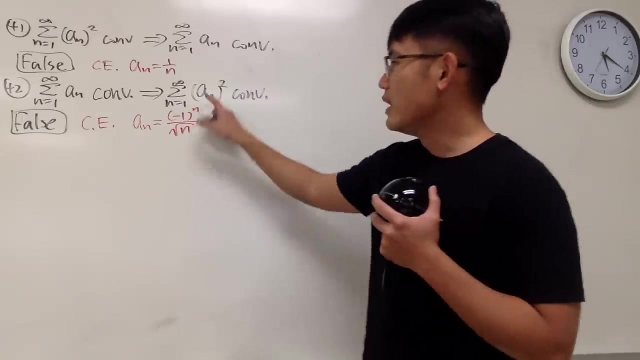 a n equals negative 1 to the nth power, which is the alternating series. okay, and then over square root of n. how's that check this out? if you put this right here, based on the alternating series test, you see 1 over square root of n is positive. 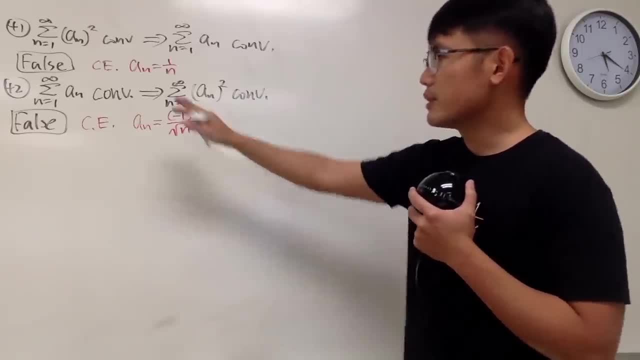 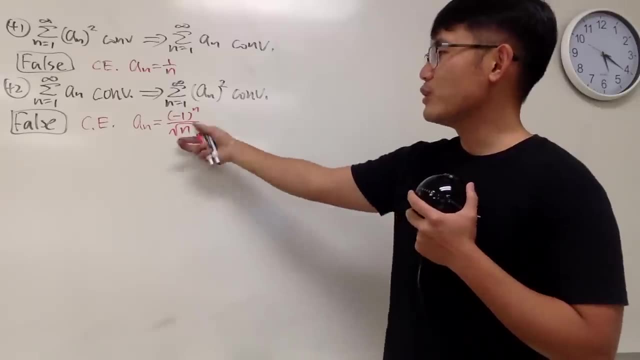 it's decreasing. and then it has limit equals 0. right, so that converges. but if you square that you kill the negative 1, you kill the alternating part, and square root of square is just n diverges. so again, this right here is false. if you have 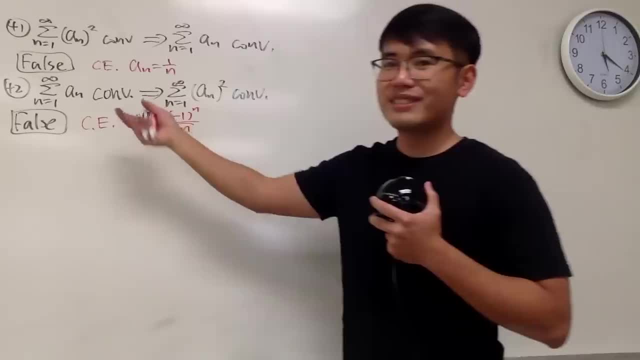 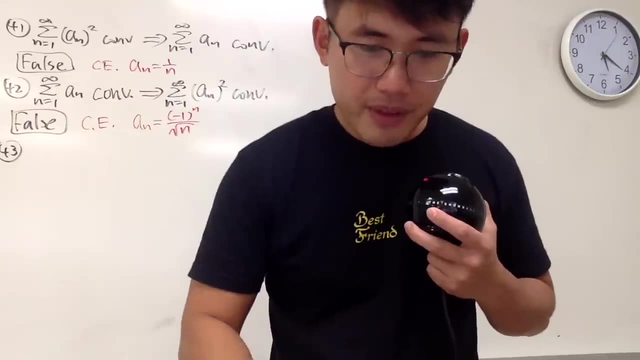 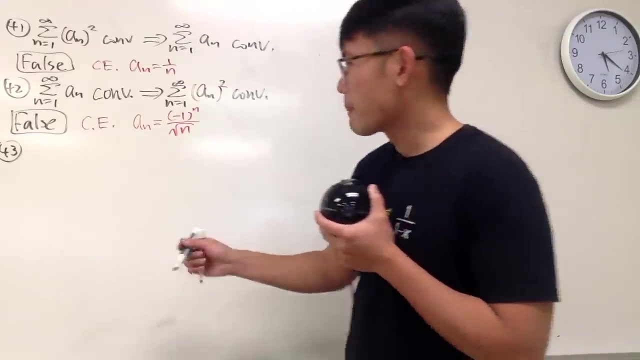 absolute value here, then you know it works, but like not this. so, but anyway, based on this statement, it's false. now number 43: if a n converges, then 1 over a n diverges. let's see. so I'll put this down: the sum as a n. 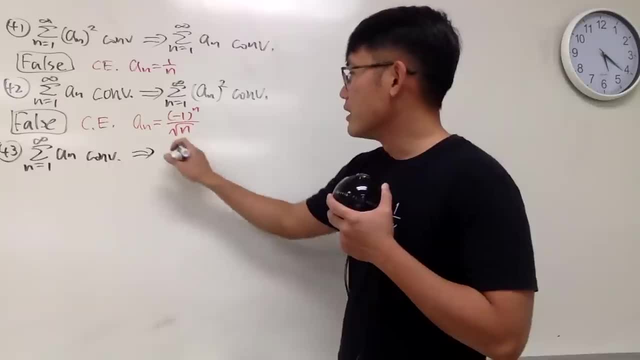 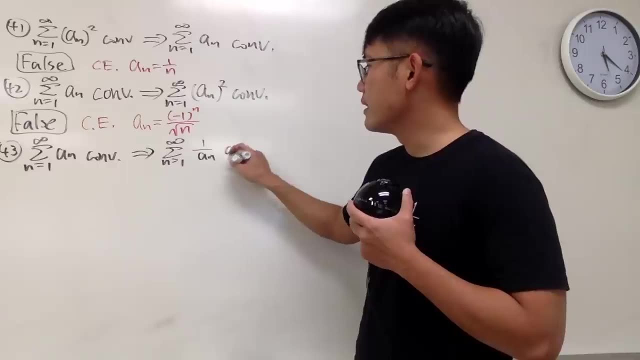 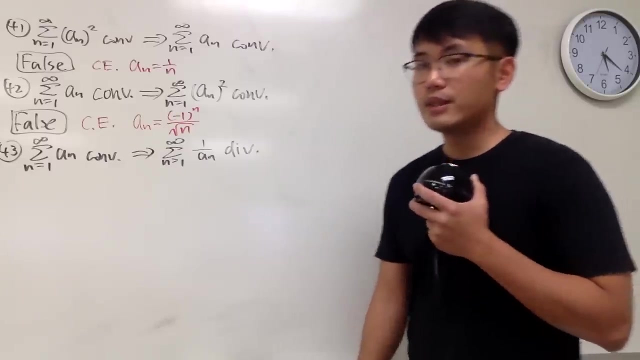 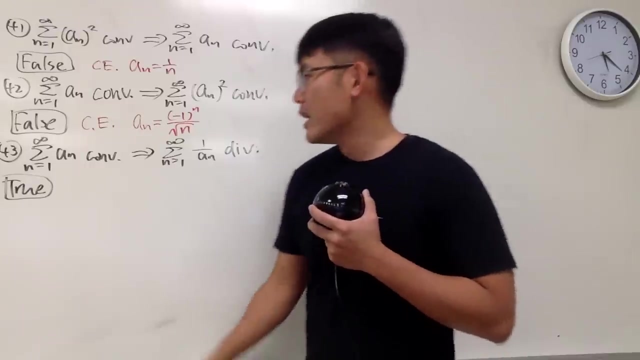 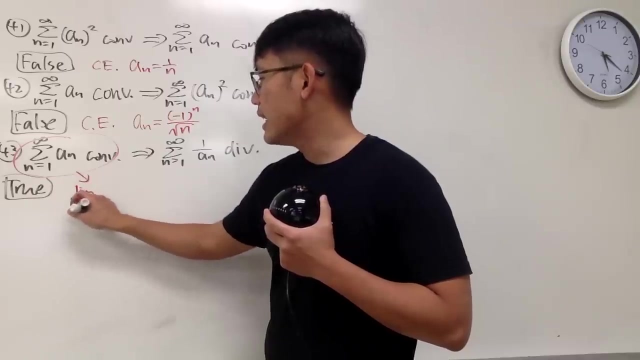 if this right here converges, does this imply the sum as n goes from 1 to infinity of 1 over a n diverges? okay, the answer to this is true. why, based on this right here, we must have the limit as n goes to infinity of a n? 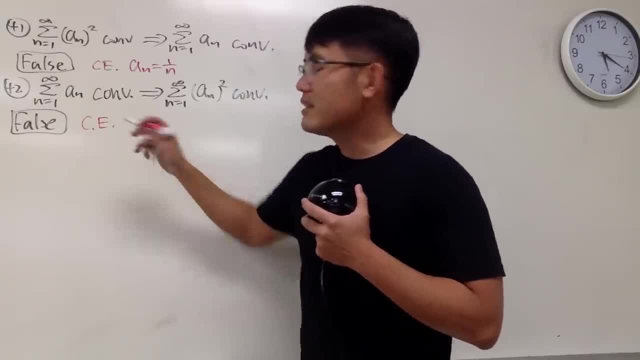 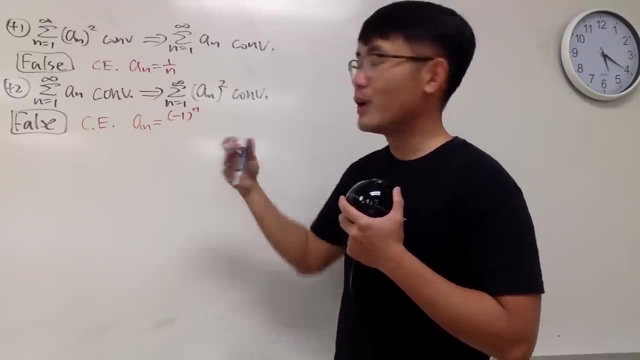 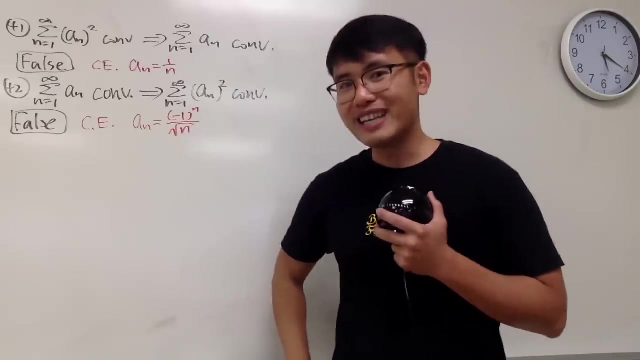 OK, I'll tell you Counter-example right here. I will just show you a: n equals negative 1 to the nth power, which is the alternating series. OK, and then over square root of n. How's that? Check this out, If you put this right here, based on the alternating series. 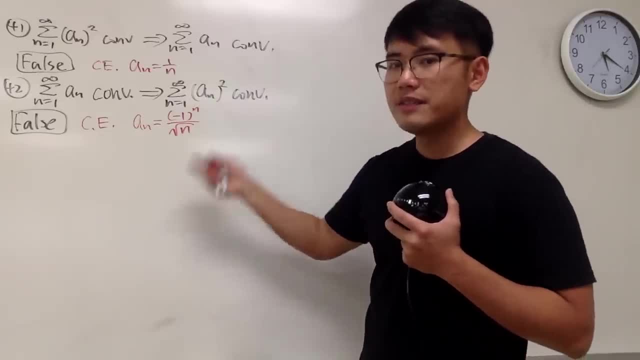 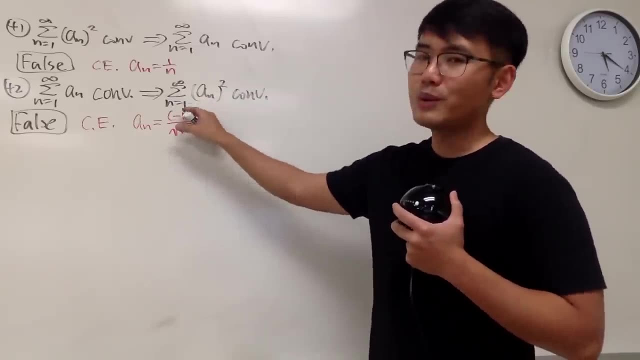 test you'll see: 1 over square root of n is positive, It's decreasing. And then it has limit equals 0, right, So that converges. But if you square that, you kill the negative 1. You kill the alternating part. 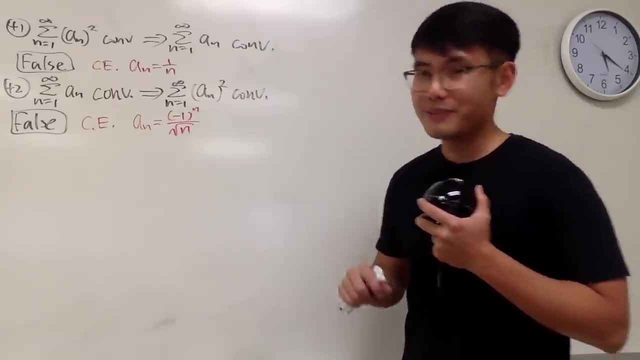 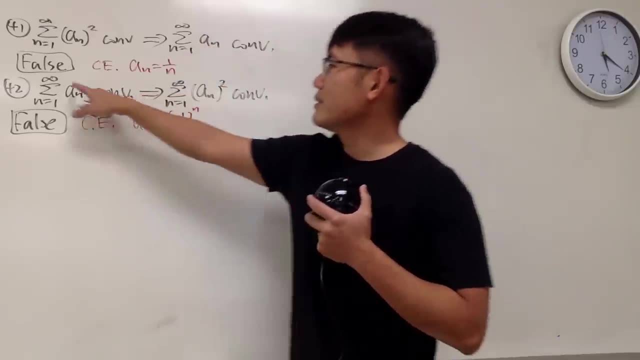 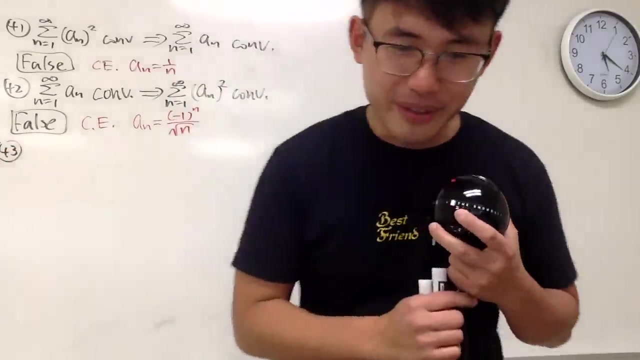 And square root of square is just n Diverges. So again, this right here is false. The truth is, if you have absolute value here, then you know it works. But like not this. So but anyway, based on this statement, it's false. Now number 43.. 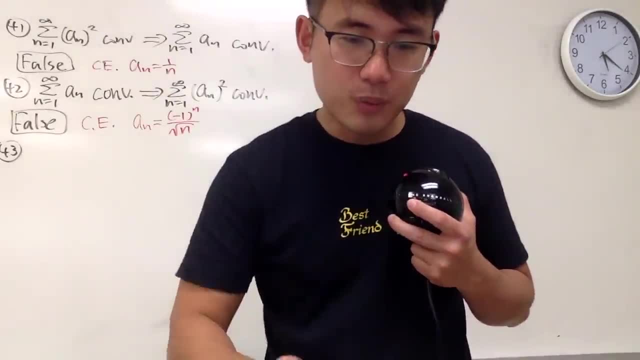 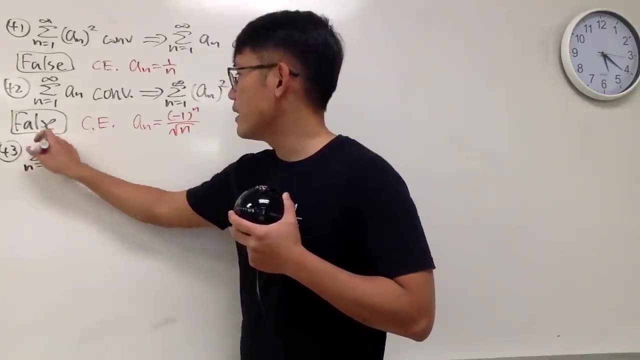 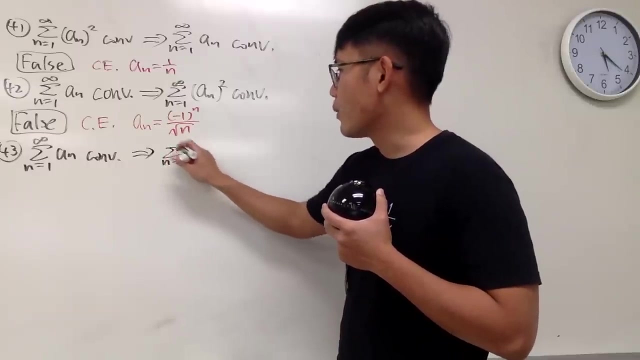 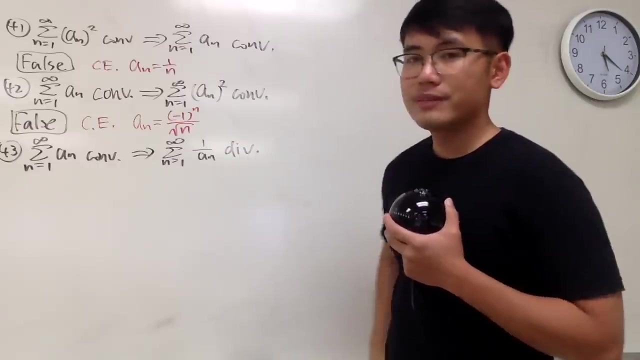 If a n converges, then 1 over a n diverges. Let's see, So I'll put this down: The sum as a n. if this right here converges, does this imply the sum as n goes from 1 to infinity, of 1 over a n diverges? 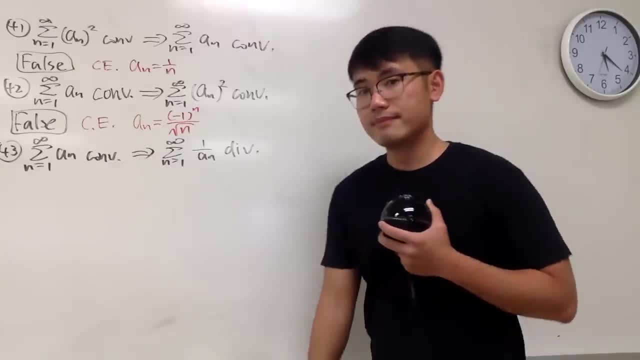 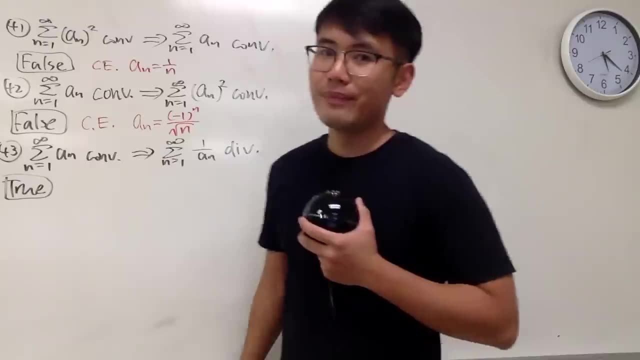 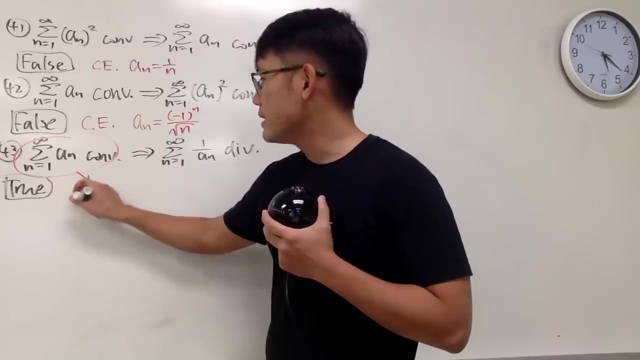 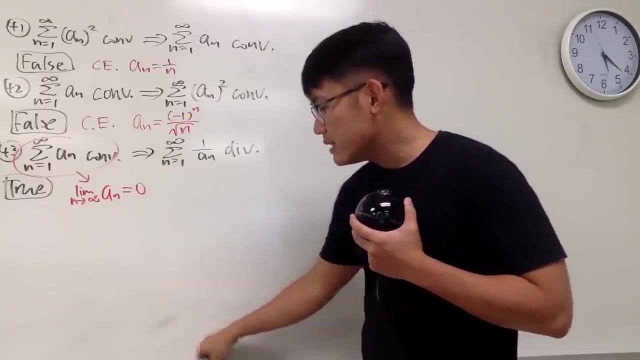 OK, The answer to this is true. Why, Based on this right here, we must have the limit- as n goes to infinity- of a n. This right here must be equal to 0. And if you take the a n, you put that in the denominator. 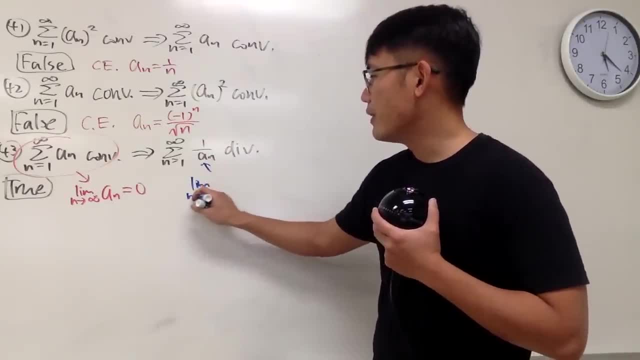 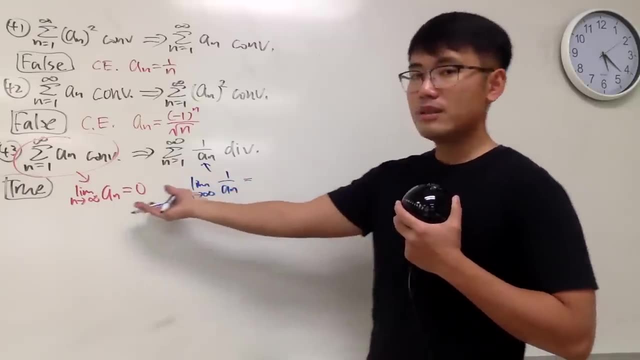 then this: right here the limit of n goes to infinity of 1 over a n. it's going to be 1 over 0, right, Because now you have that in the denominator: It's going to be 1 over 0.. 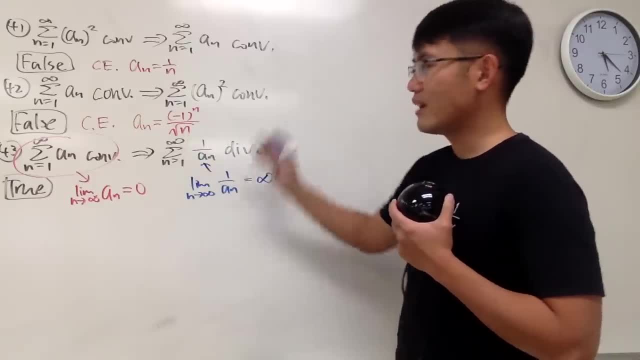 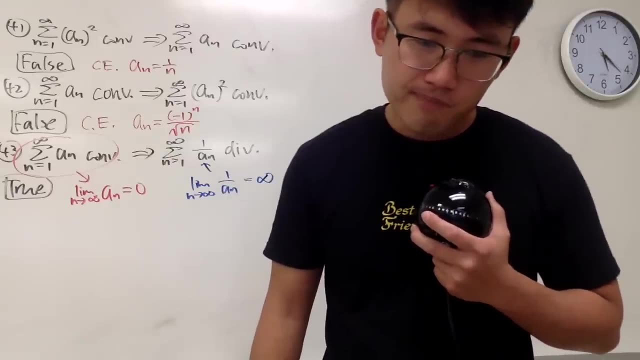 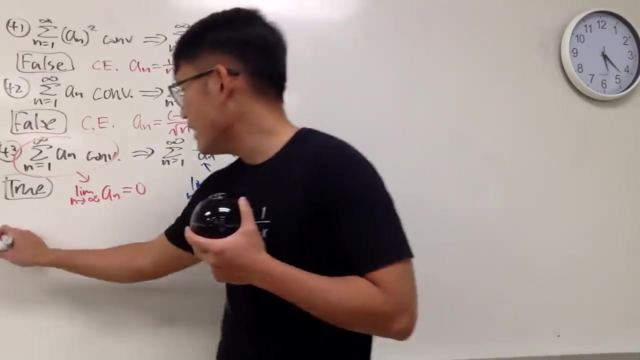 This is going to be really bad. So of course, this right here diverges. So this is true, OK. Next we have: hmm, OK, How about the other way around, If I say number 44, right, Let's see. 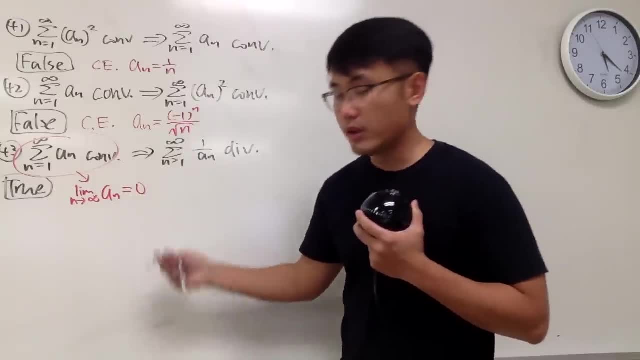 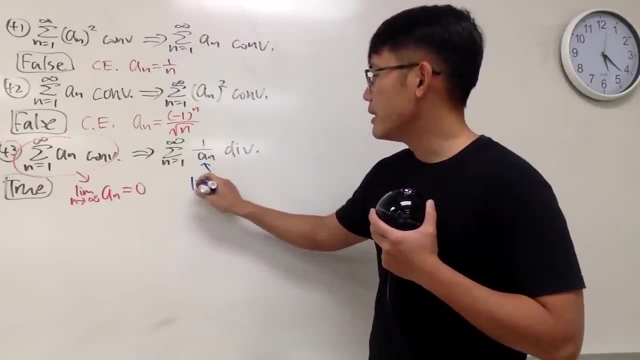 this right here must be equal to 0, and if you take the a n, you put that in the denominator, then this right here, the limit of n goes to infinity of 1 over a n. it's going to be 1 over 0, right, because now you have that. 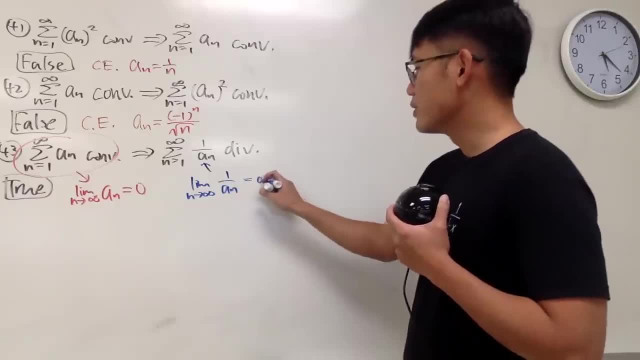 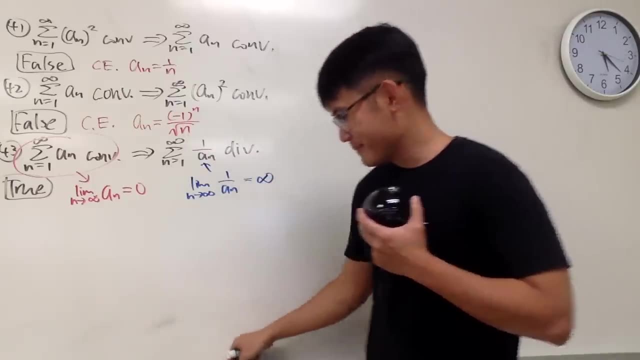 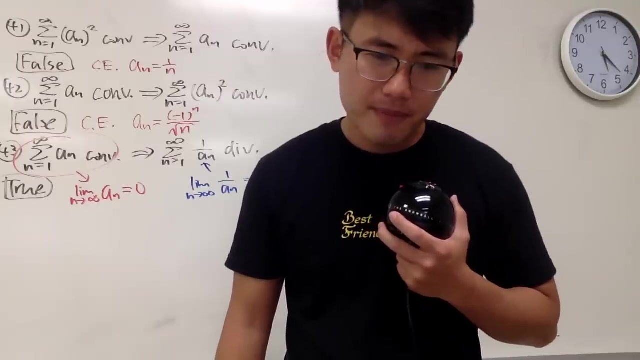 in the denominator, it's going to be 1 over 0. this is going to be really bad, so of course, this right here diverges. so this is true, okay. next we have: hmm, let's see, let's see, hmm, okay, how about the other way around? 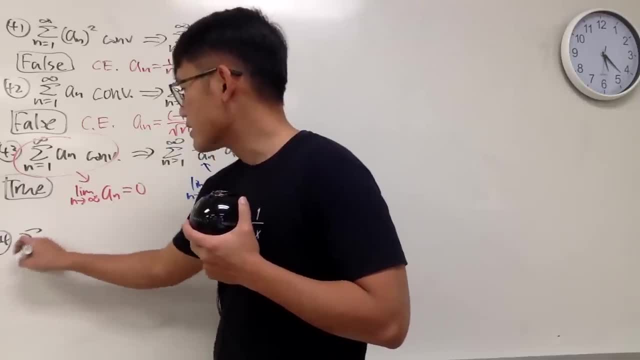 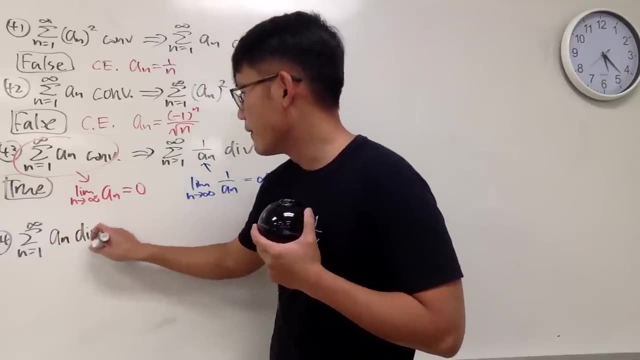 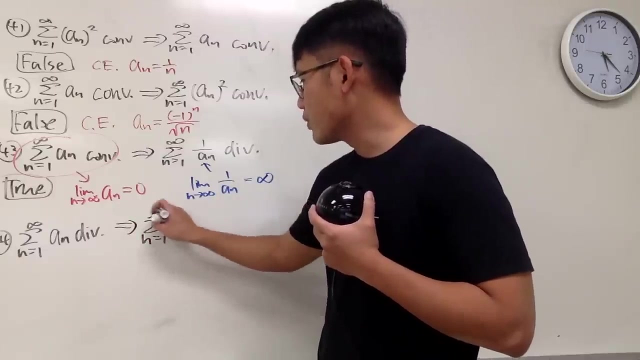 if I say number 44, right. let's see if we say the sum as n goes from 1 to infinity and suppose a n diverges, a n diverges and we want to show that if the sum as n goes from 1 to infinity, 1 over a n. 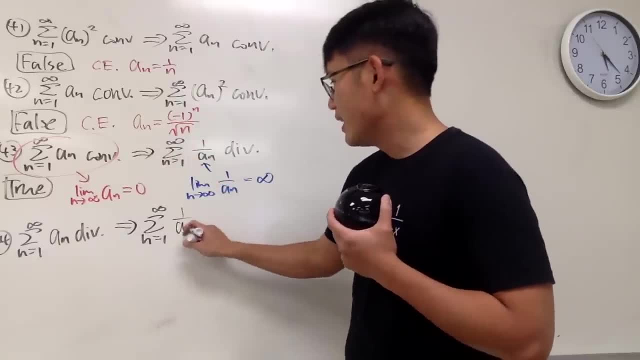 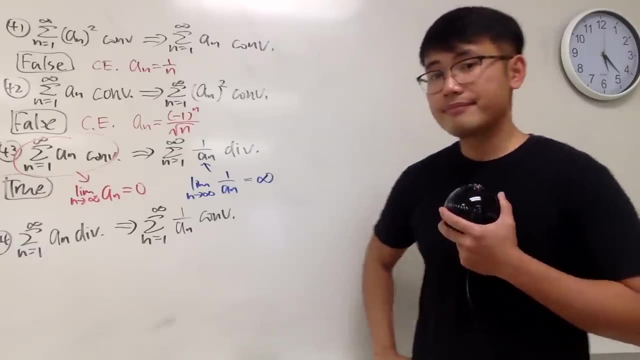 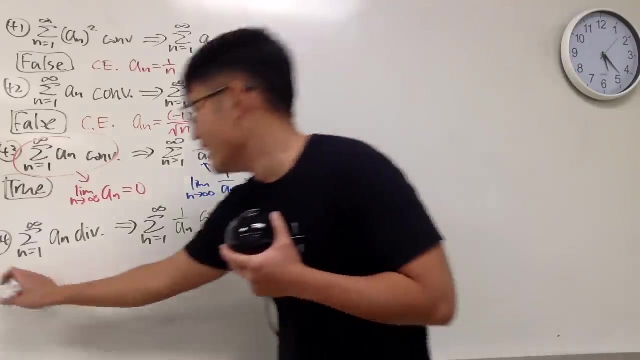 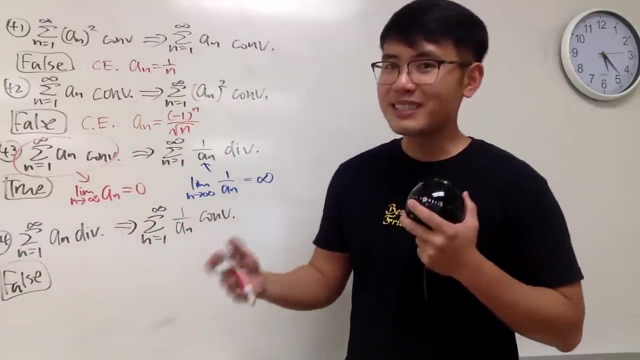 so it's just like a ref, it's just like a converse statement: a- n does this converge? hmm, false right? this right here is false. why keep in mind of some of the you know classic examples of divergence in this case? I will just tell you counter example. 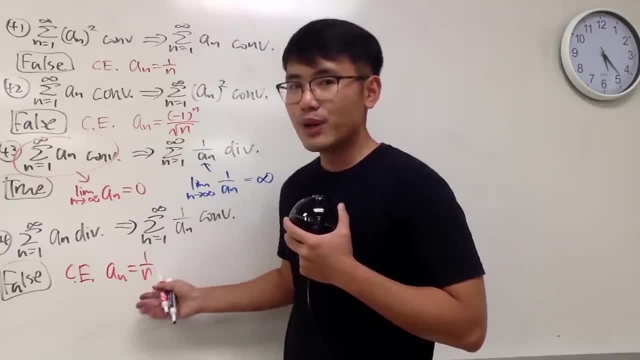 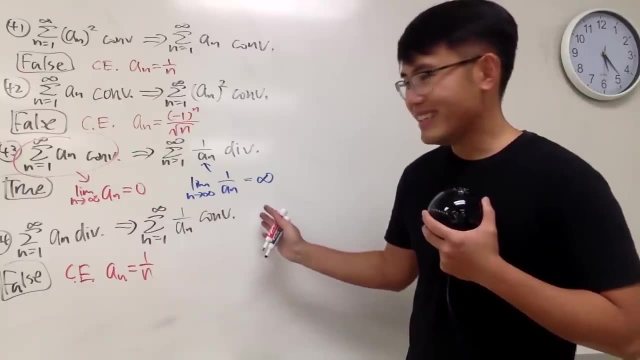 we take a n to be 1 over n, as we all know. if you put it right here, that diverges. if you do the reciprocal, the sum of n, all the natural numbers- does not converge. please don't say negative 1 over 12 if you're still watching. 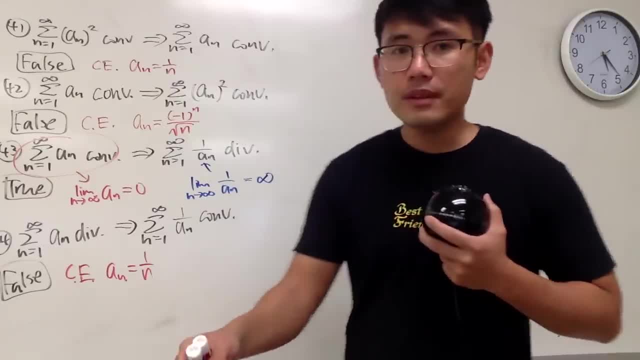 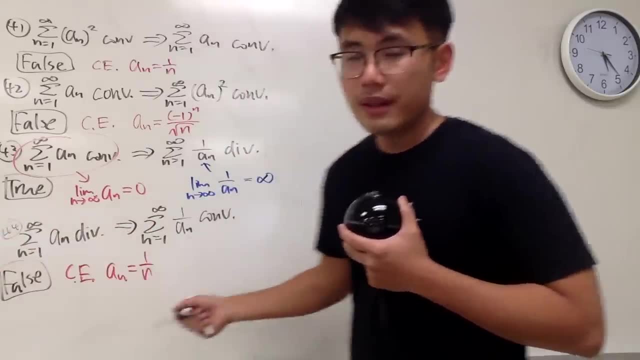 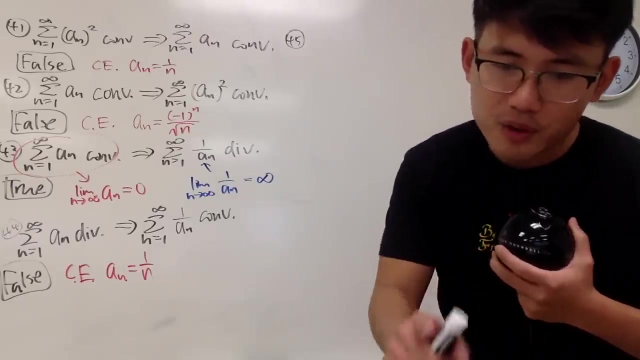 don't say that. anyway that right here. hmm, that's number 44. but like, anyway this right here, it's false. the other one was true, though, right. so yeah, we are going to do: if a n converges, then a n divided by n, the series for that. 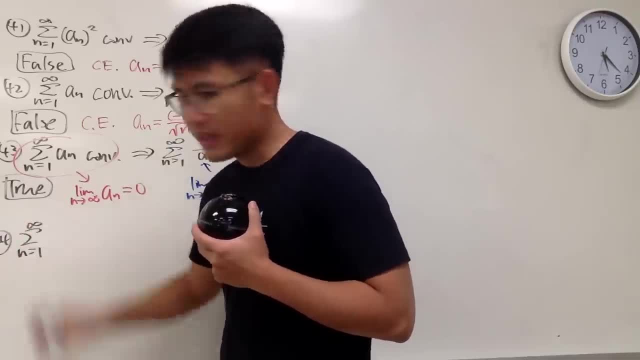 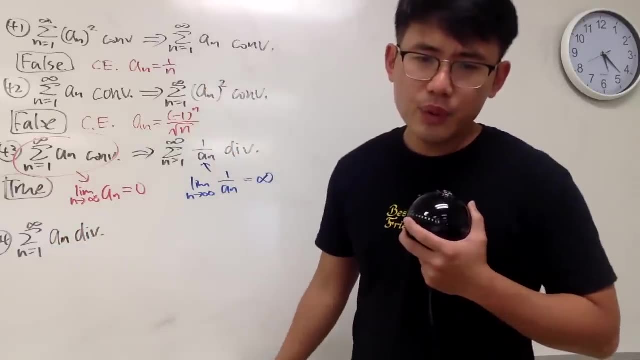 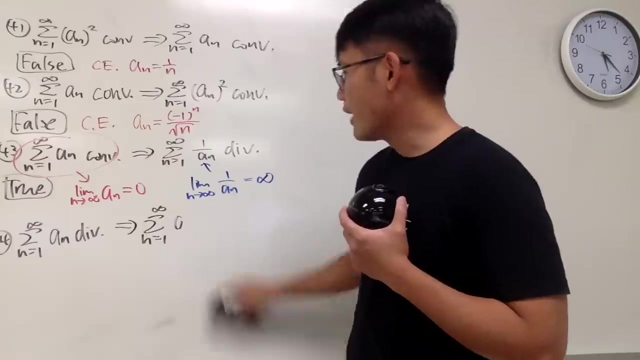 If we say the sum as n goes from 1 to infinity and suppose a n diverges, a n diverges. And we want to show that if the sum as n goes from 1 to infinity, 1 over a n, So it's just like a, it's just like a conference statement. 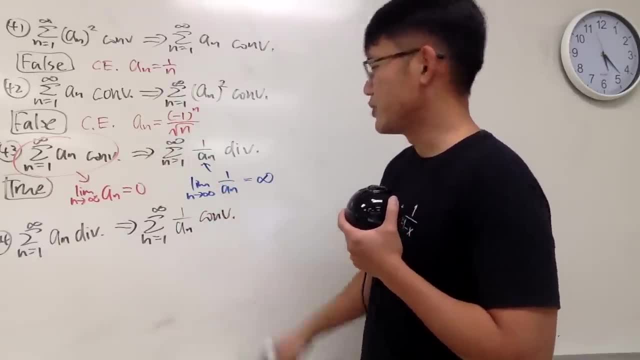 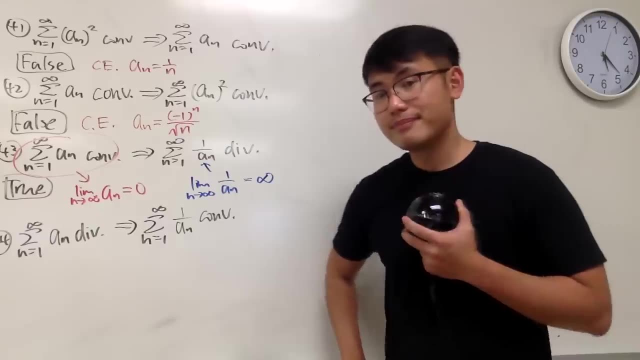 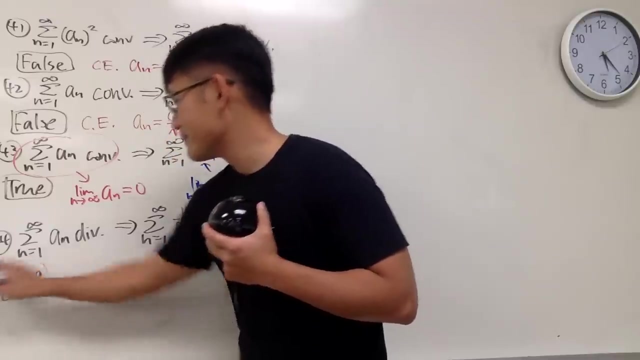 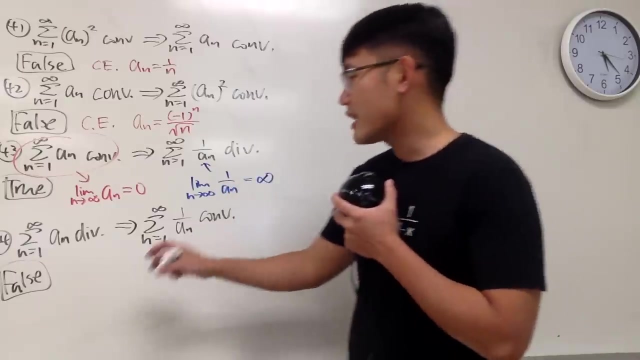 a n. does this converge? Hmm, False Right. This right here is false. Why Keep in mind of some of the you know classic examples of divergence In this case? I will just tell you counter example. We take a n to be 1 over n. 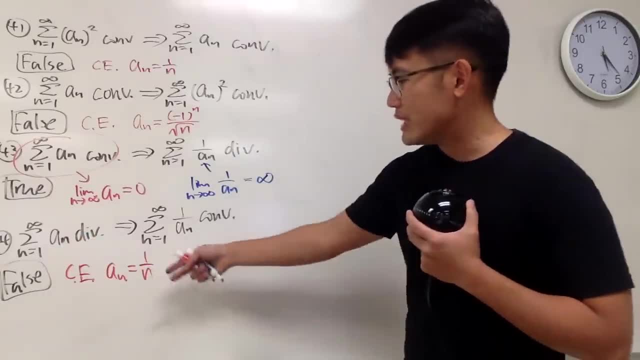 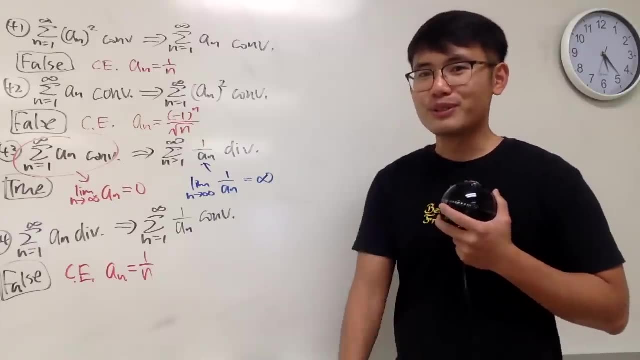 As we all know. if you put it right here, that diverges. If you do the reciprocal, the sum of n- all the natural numbers- does not converge. Please don't say negative 1 over 12.. If you're still watching, don't say that. 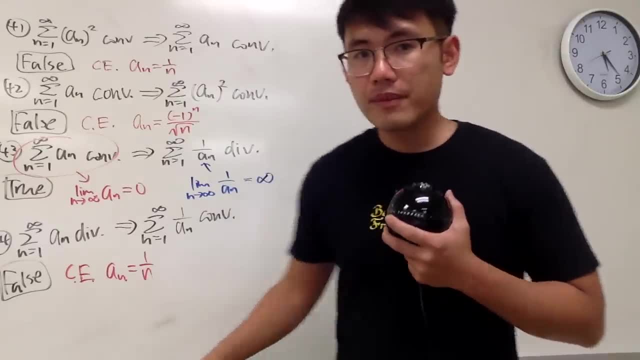 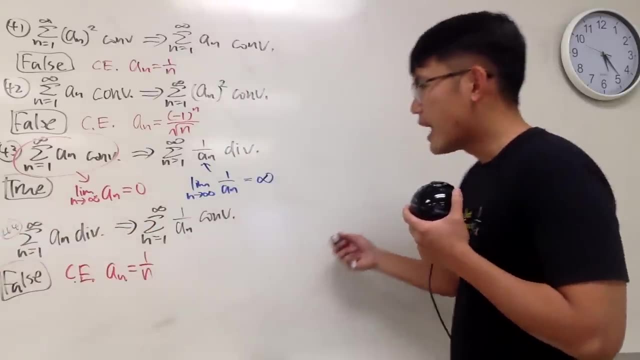 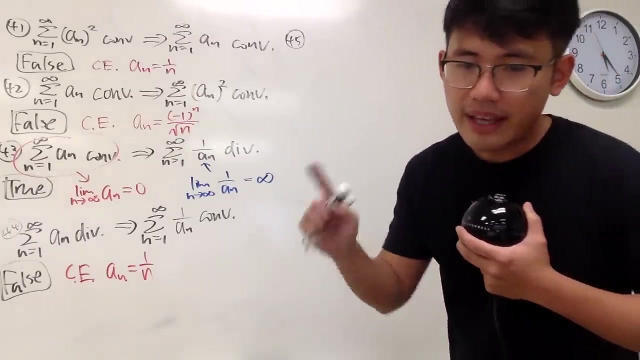 Anyway, that right here, that's number 44. But like, anyway, this right here is false. The other one was true though. So yeah, Now number 45. We are going to do: if a n converges, then a n divided by n, the series for that. 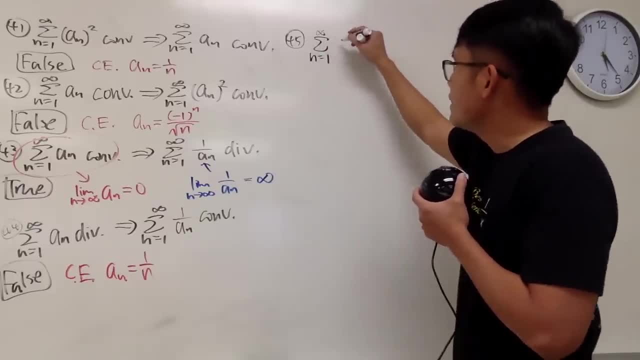 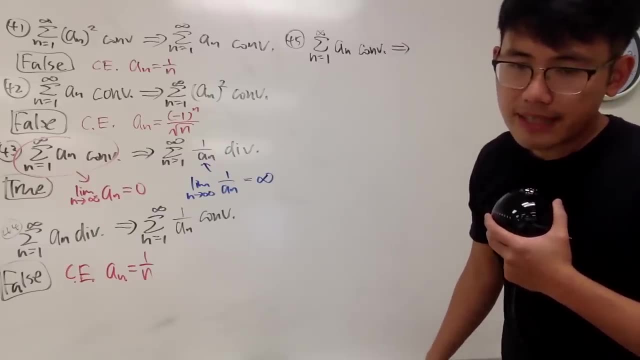 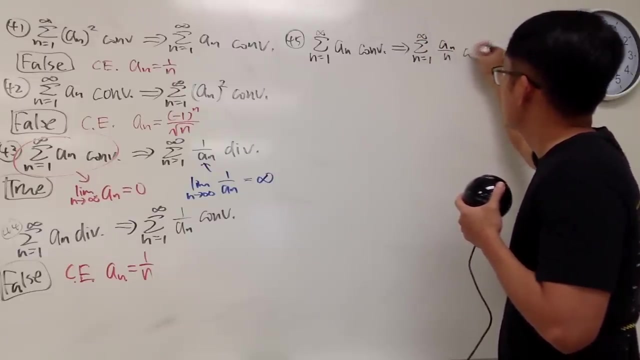 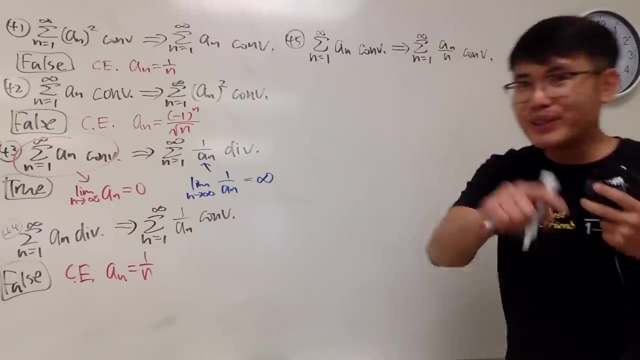 let's see, does that converge or not? n goes from 1 to infinity. a n. If this right here converges, then let's see: Hmm, Does this imply that a n over n? This right here is true? So let me just tell you guys why. 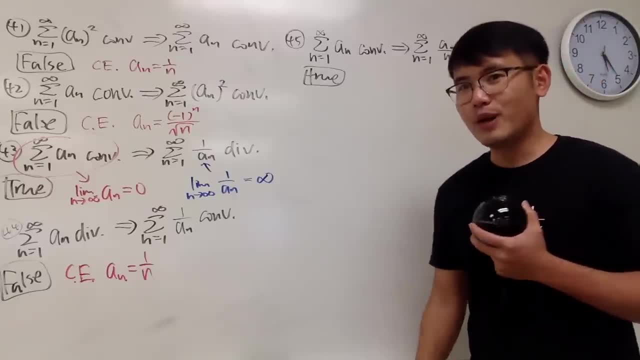 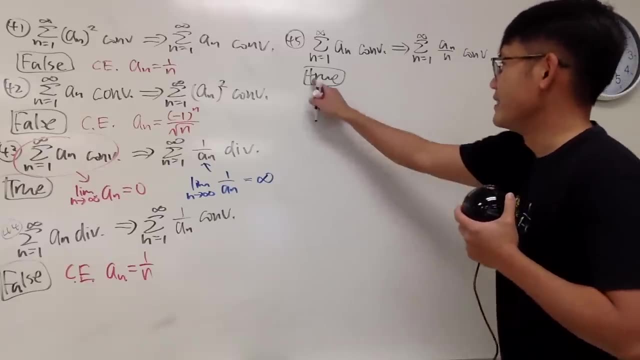 And maybe you guys can leave a comment down below to see if you are a Cal2 teacher, do you give like true-false questions? or if you are a Cal2 student, does your teacher give you true-false questions? But I certainly will. 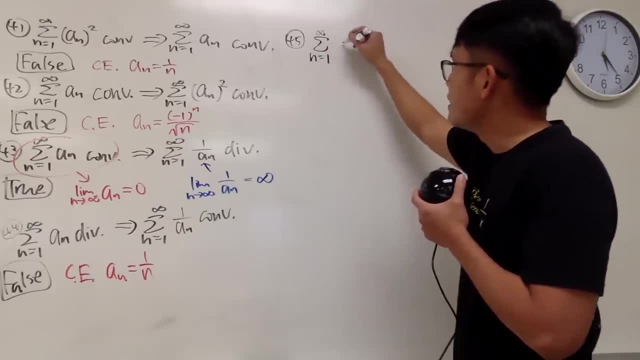 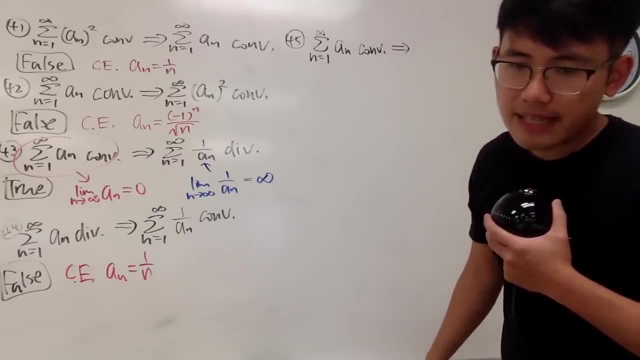 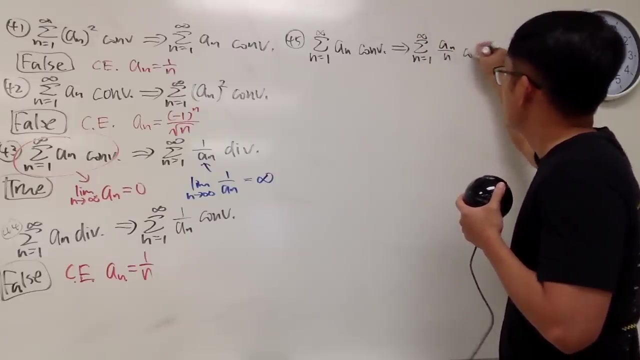 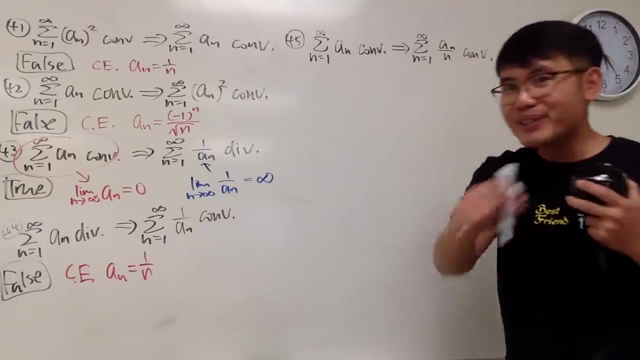 let's see, does that converge or not? n goes from 1 to infinity. a n. if this right here converges, then let's see: hmm, does this imply that a n over n- this right here is true? so let me just tell you guys why, and maybe you guys can. 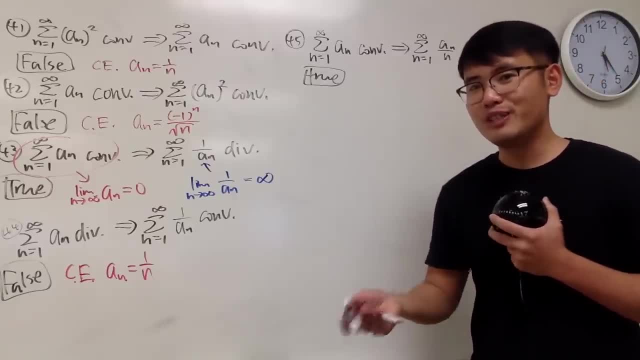 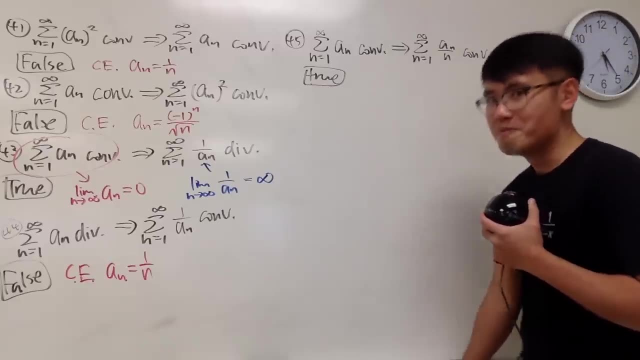 leave a comment down below to see if you are a calc 2 teacher, do you give like true false questions? or if you are a calc 2 student, does your teacher give you true false questions? but I certainly will. so if you guys are watching from my class, 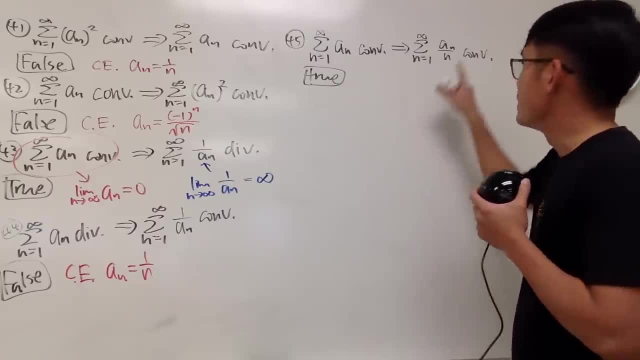 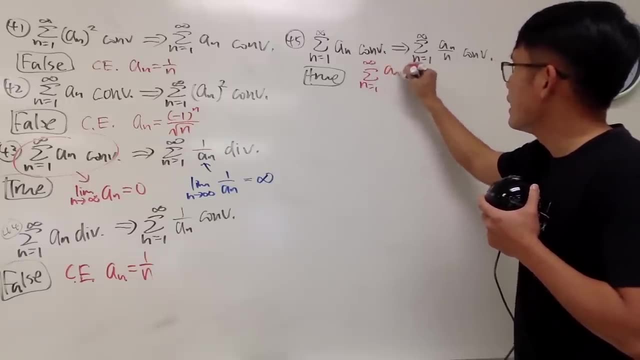 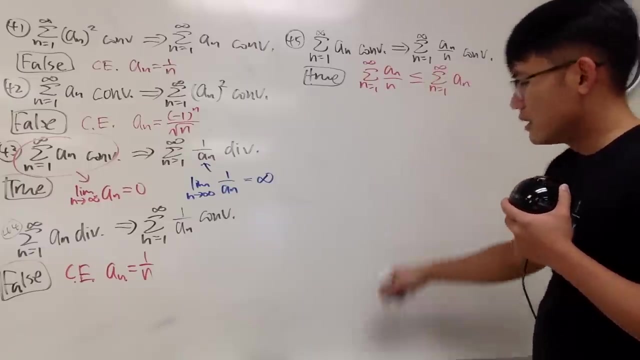 you guys know how to study. okay, anyway, this right here is true. why? because you can see that you can show that the sum as n goes from 1 to infinity of a n over n, this right here is less than or equal to that, of course. why? 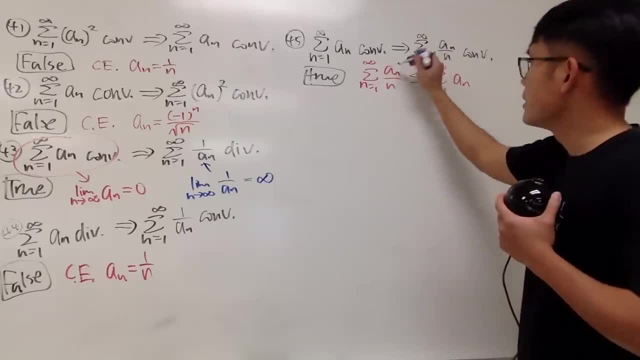 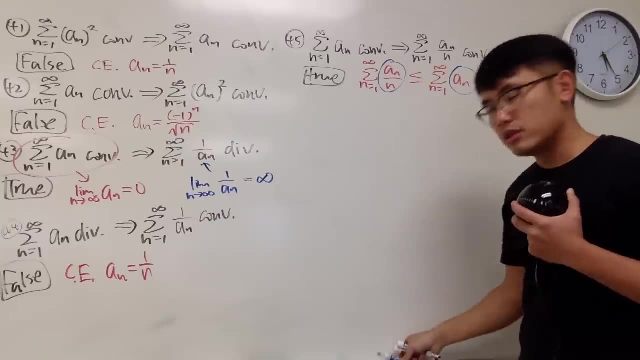 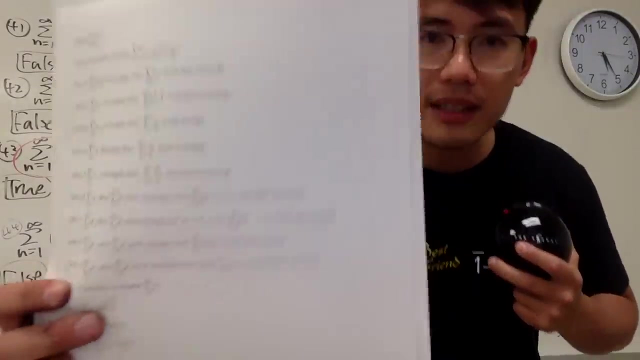 because the denominator is bigger. if you guys look at the denominator right here, this right here is of course bigger than the denominator is bigger. so that means the whole fraction is going to be smaller than that. so this right here is true. now continue if you see both. 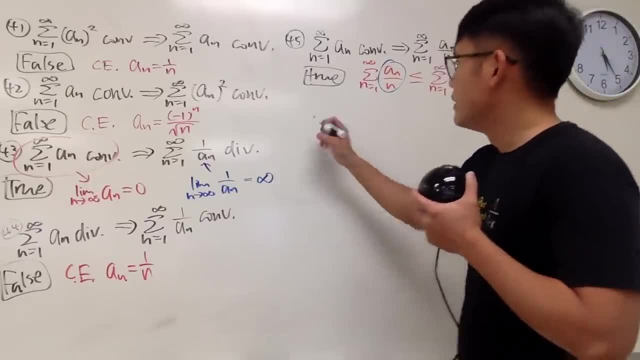 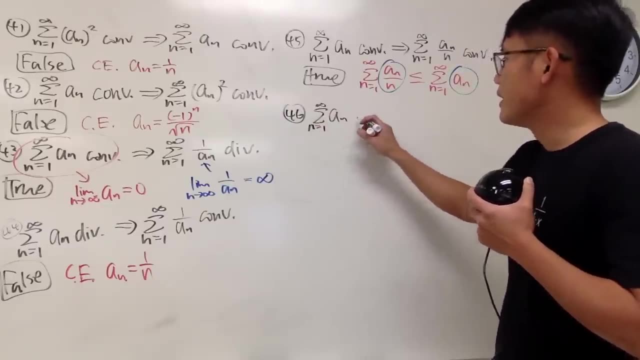 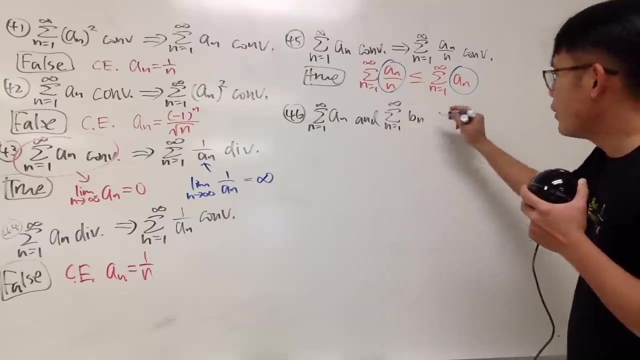 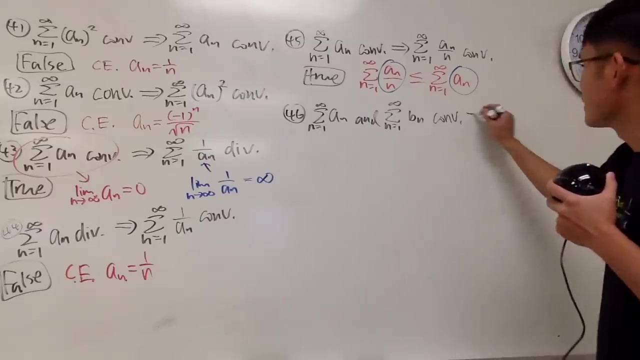 of them converge? do they converge when you add, let's see number 46. so the series of a, n, n goes from 1 to infinity and the series of b, n, like this. suppose both of them converge, does that imply? well, I'll just actually put down the sum. 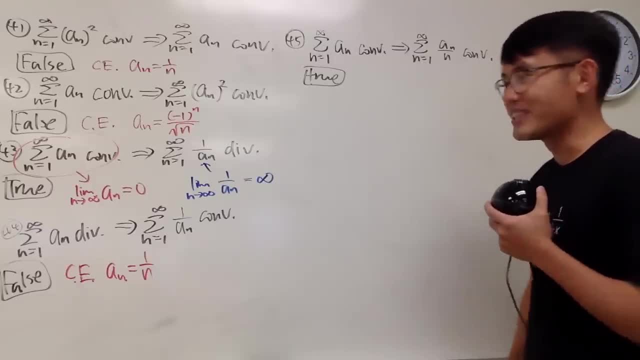 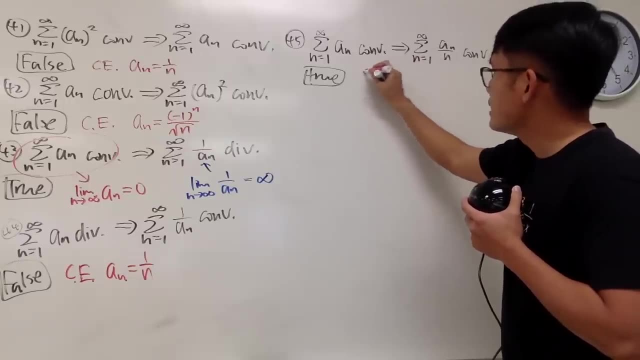 So if you guys are watching from my class, you guys know how to study, okay. Anyway, this right here is true Why? Because you can see that you can show that the sum as n goes from 1 to infinity of a n over n. 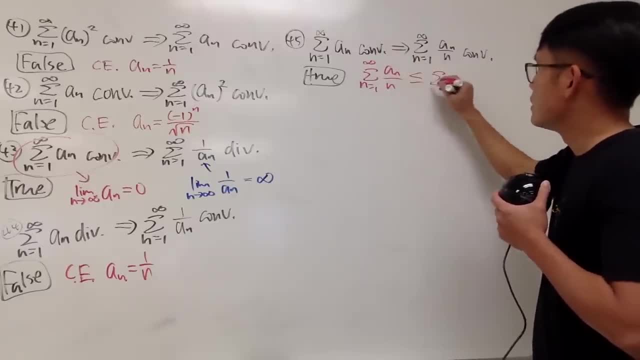 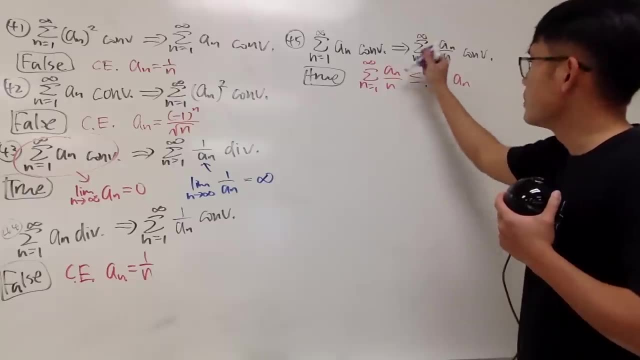 this right here is less than or equal to that, of course. Why? Because the denominator is bigger. If you guys look at the denominator right here, this right here is of course bigger than the denominator is bigger. so that means the whole fraction is going to be smaller than that. 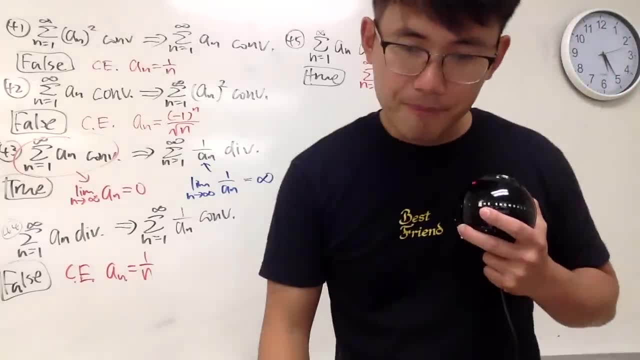 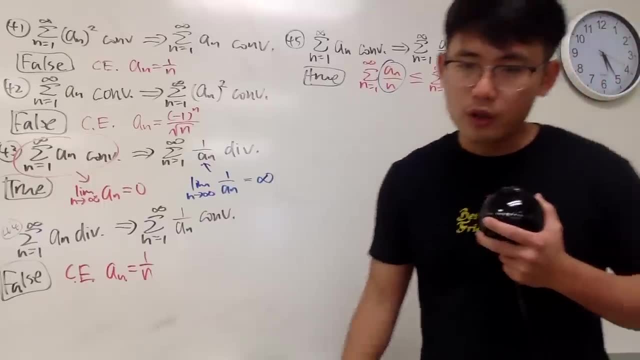 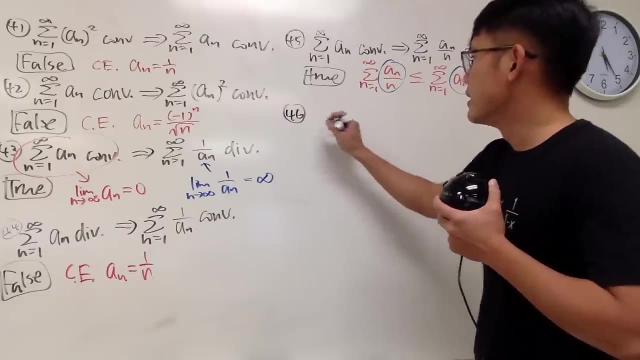 So this, right here, is true. Now continue: If the series of a n and series of b n, if they both converge, do they converge when you add? Let's see Number 46.. So the series of a- n. 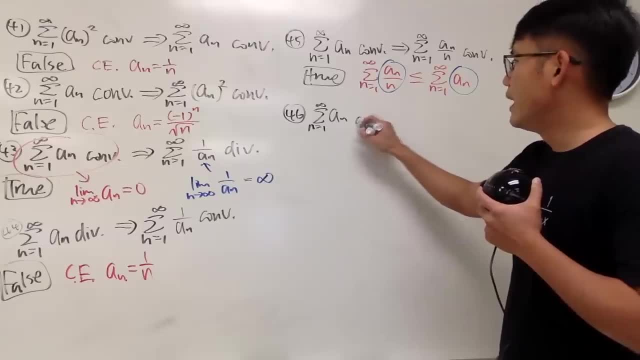 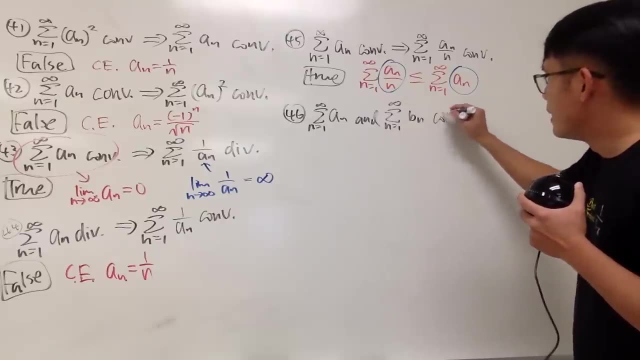 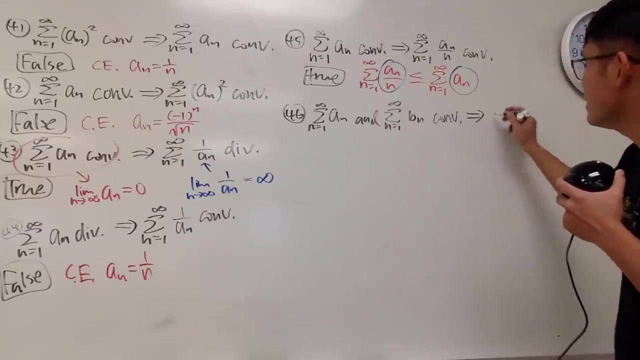 n goes from 1 to infinity and the series of b? n like this: suppose both of them converge, does that imply? well, just actually put down the sum right here, put down the implication right here. does that imply when we do this? 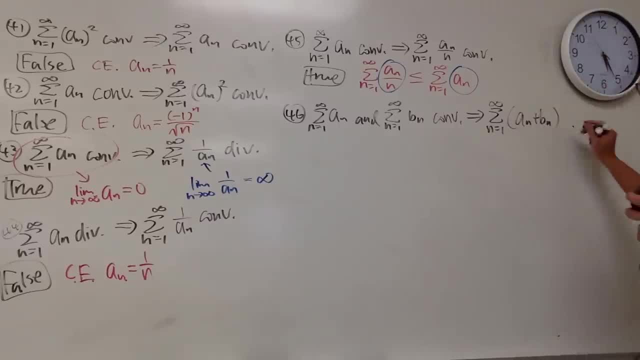 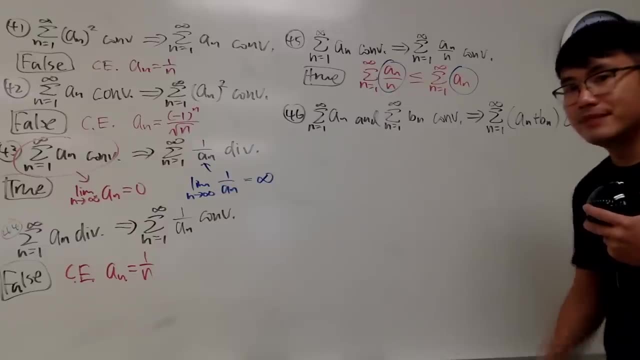 a, n plus b? n, do we also get convergent right here. So what do you guys think? This right here is true, Very true, Very, very true. So let me just write this down right here for you guys. 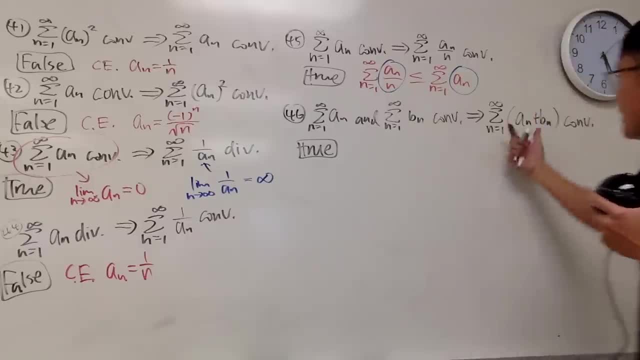 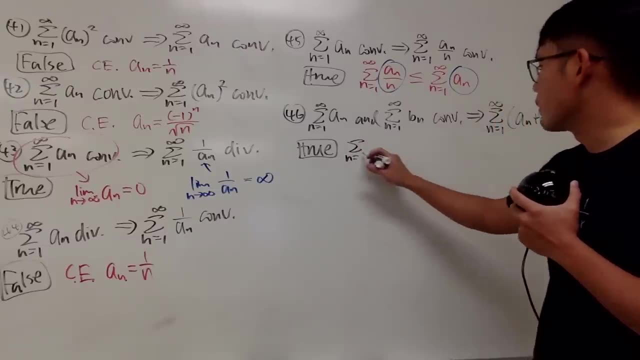 This is very true. Why? Because when you are talking about the sum of this and that all we can do is, of course, we can just write this down as the sum, as n goes from 1 to infinity of a n. 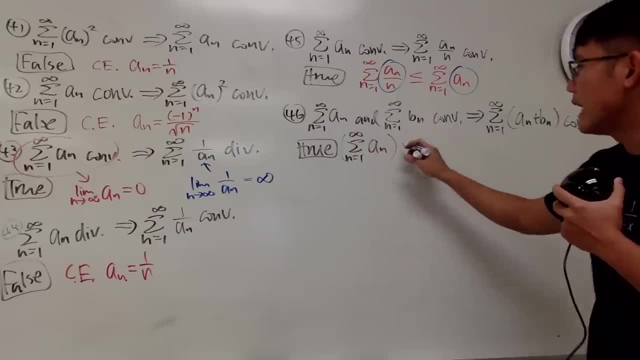 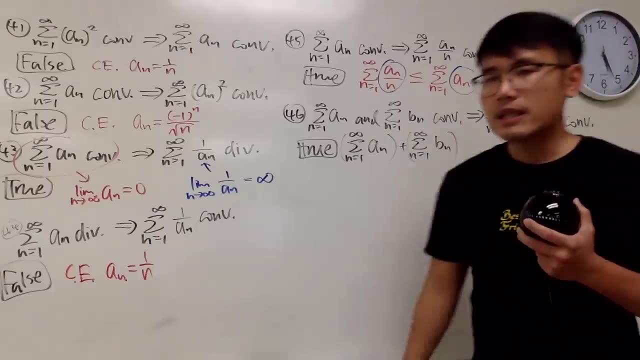 especially if they are convergent, and then you can just add the sum, as n goes from 1 to infinity- of b, n, and of course you will also have to consider some like conditional convergence whatsoever. The idea of the conditional convergence is that 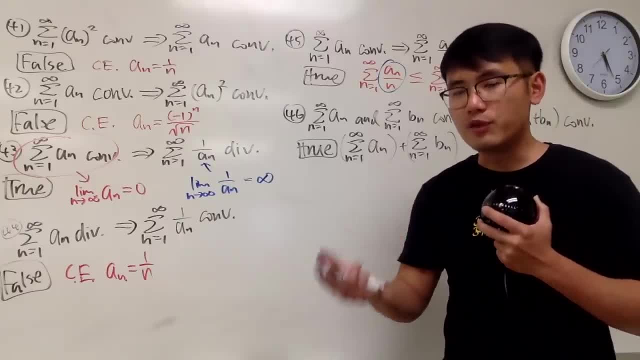 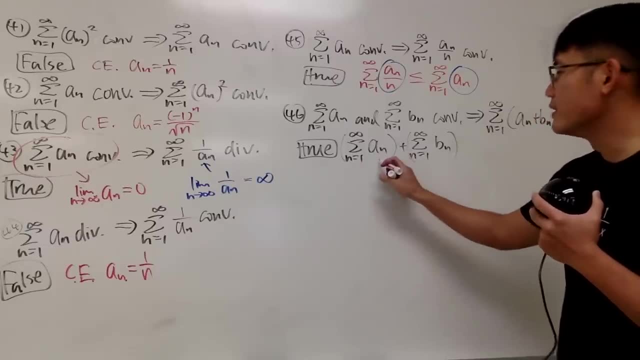 if you rearrange the terms, you may end up with a different sum, But it doesn't really matter, because this right here is finite. this right here is also finite. so I'll just tell you: this is less than infinity. this right here is also less than infinity. 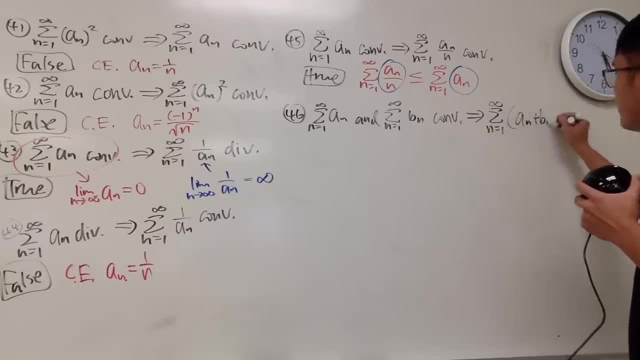 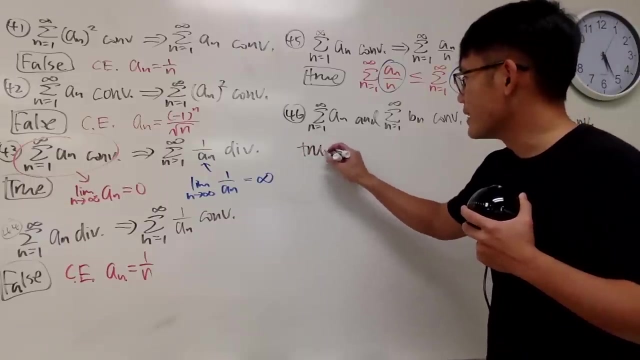 right here. Do this: a n plus b? n. do we also get convergent right here? So what do you guys think? This right here is true, very true, very, very true. So let me just write this down right here for you guys: 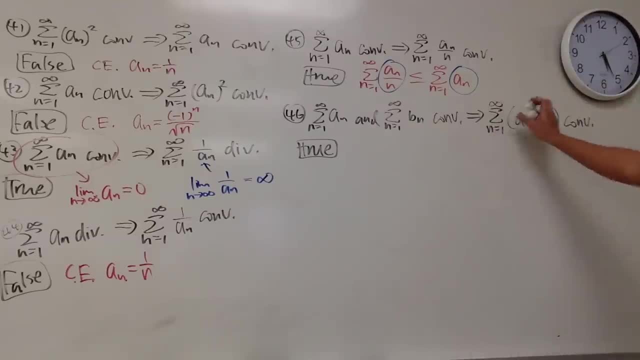 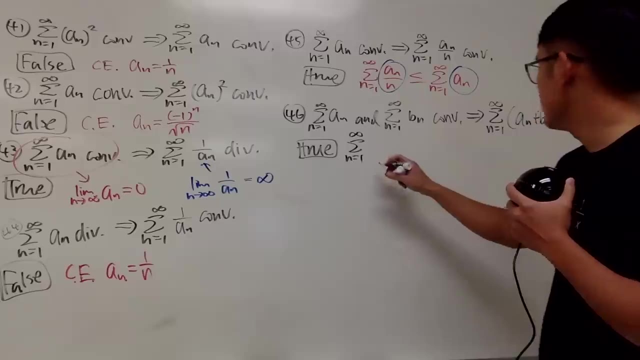 This is very true. Why? Because when you are talking about the sum of this and that all we can do is, of course, we can just write this down as the sum, as n goes from 1 to infinity of a n, especially if they are convergent. 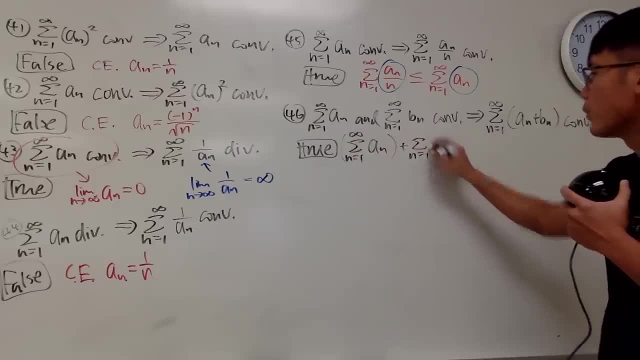 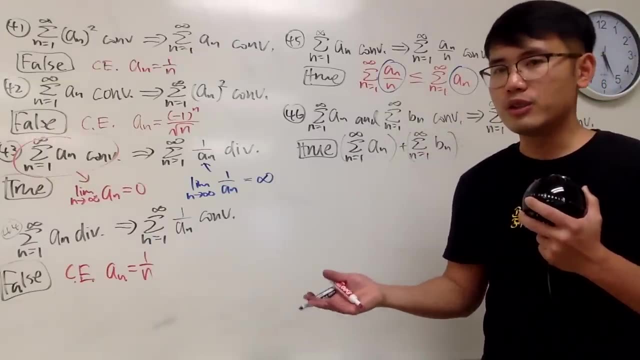 And then you can just add the sum, as n goes from 1 to infinity, of b, n, And of course you will also have to consider some like a conditional convergence whatsoever. The idea of the conditional convergence is that if you rearrange the terms, 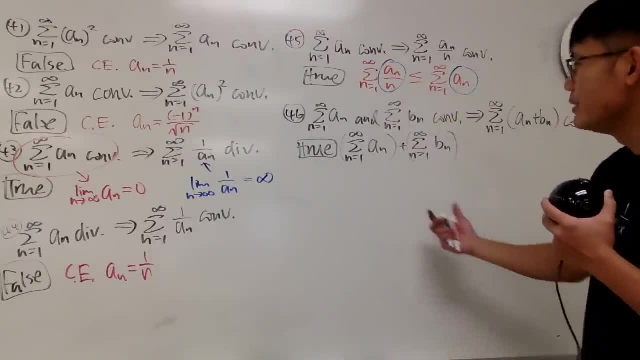 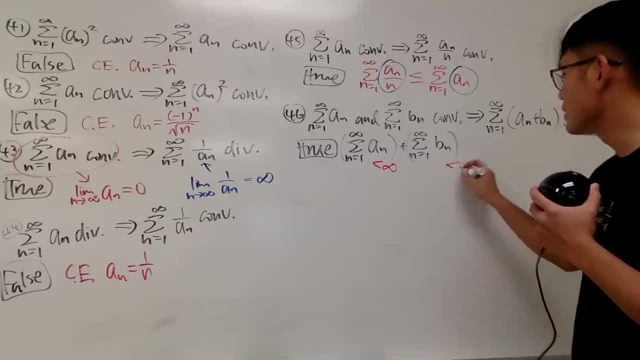 you may end up with a different sum, But it doesn't really matter, because this right here is finite. This right here is also finite. So I'll just tell you: this is less than infinity. This right here is also So less than infinity. 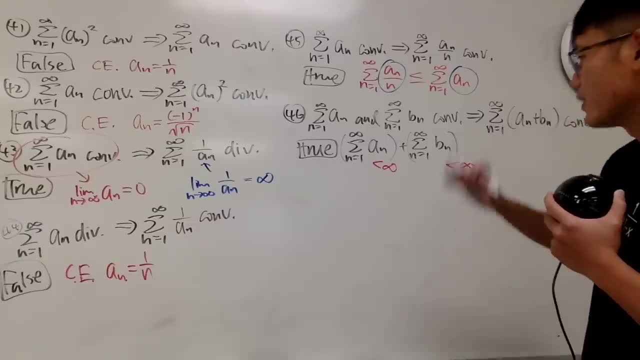 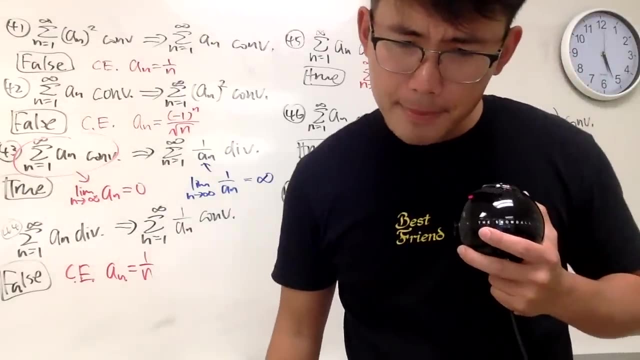 A finite plus finite number is also, of course, less than infinity. So we are done for sure, We are good for sure. Number 47.. Hmm, If the series of a? n and the series of b? n both diverge, how about if we subtract them? 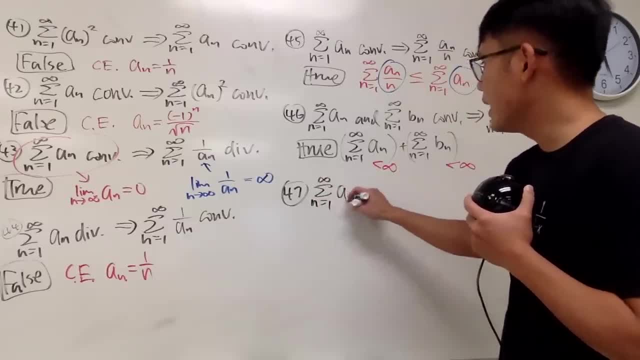 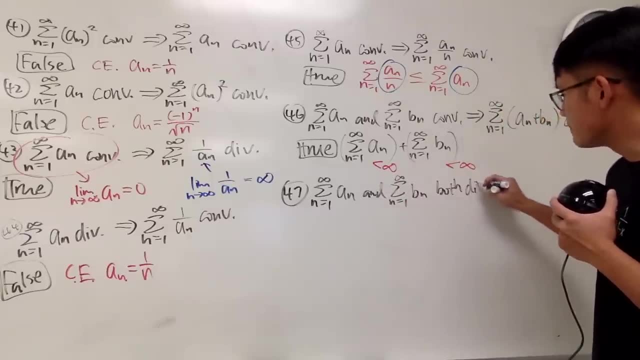 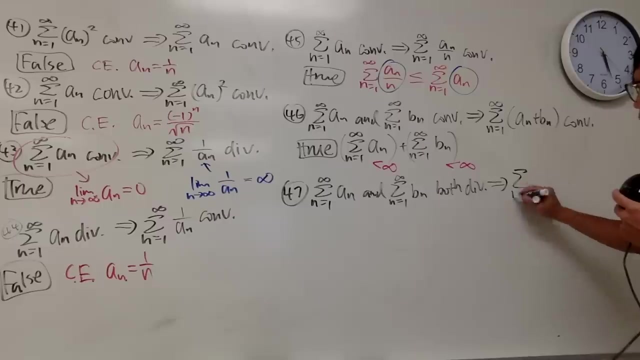 Let's see If the series of n goes from 1 to infinity a n and the series of n goes from 1 to infinity b n both diverges, right? If they both diverges, hmm, how about if we subtract them? and it goes from 1 to infinity of a n minus b n. 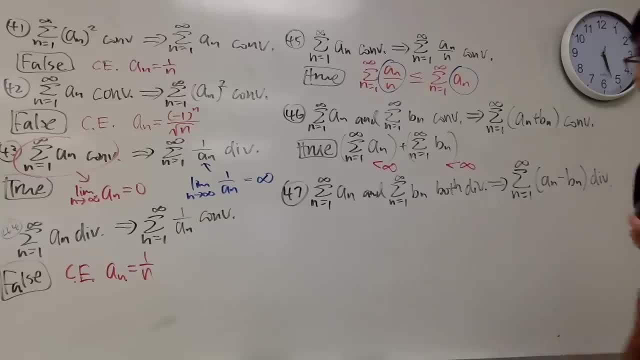 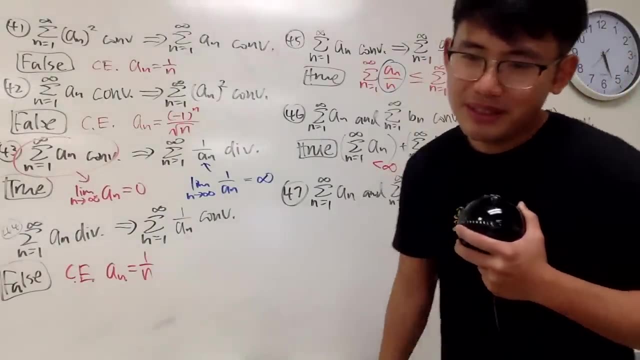 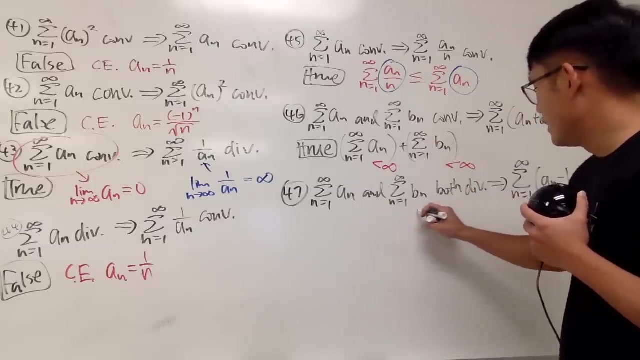 Does this also have to diverge as well? And to make this more fun, I will also add a little condition. okay, I will just say: and a, n is not the same as b? n, Otherwise you can just put that 1 over n and 1 over n. 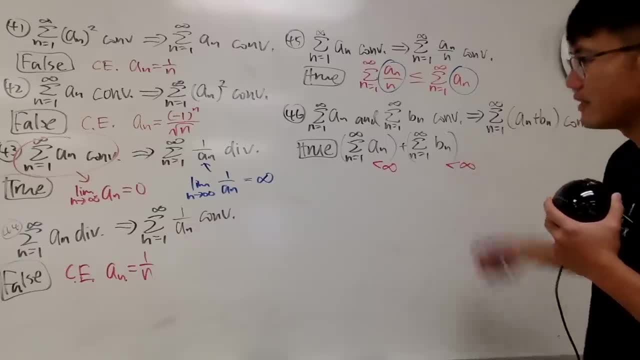 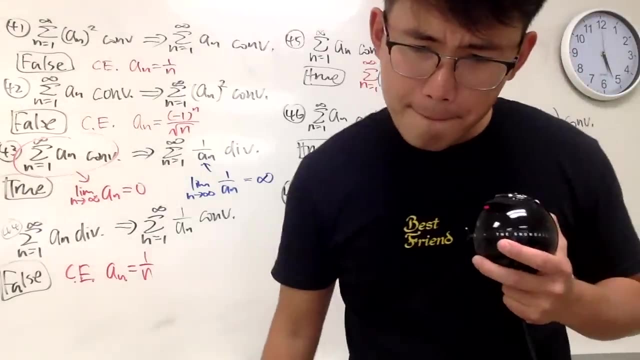 a finite plus finite number is also, of course, less than infinity. so we are done for sure. Well, good For sure. Number 47.. Hmm, If a, if the series of a- n and the series of b- n both diverge. 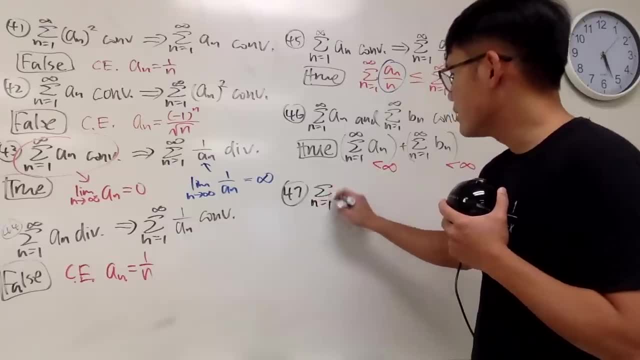 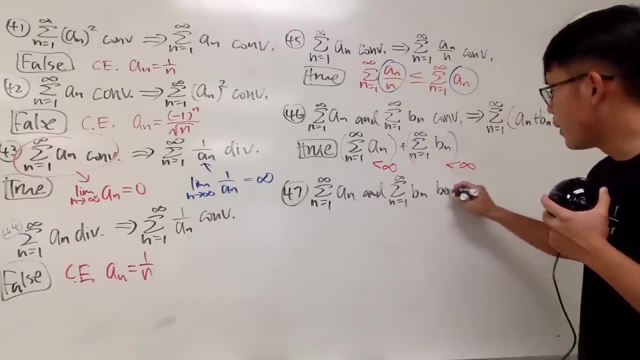 how about if we subtract them? Let's see If the series of n goes from 1 to infinity a, n and the series of n goes from 1 to infinity b, n, both diverges. right if they both diverges. 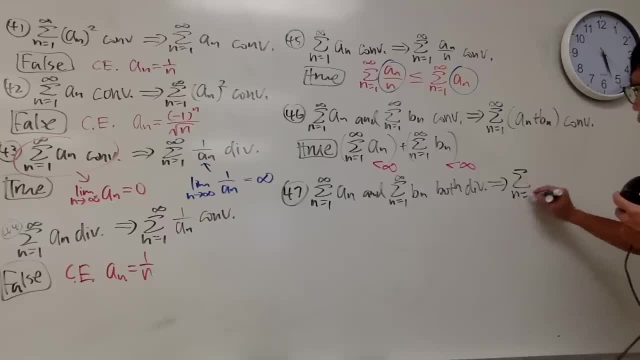 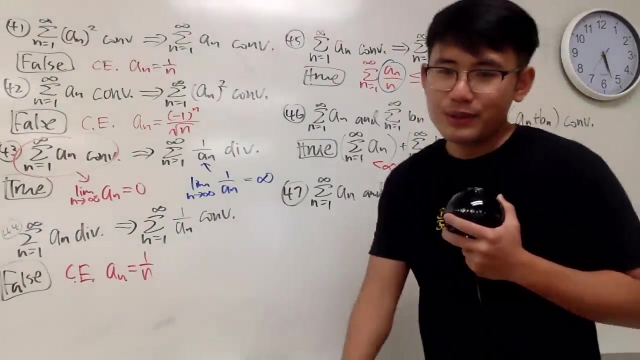 hmm, how about if we subtract them? n goes from 1 to infinity of a n minus b n. does this? does this also have to diverge as well? And to, to make this like, to make this more fun. 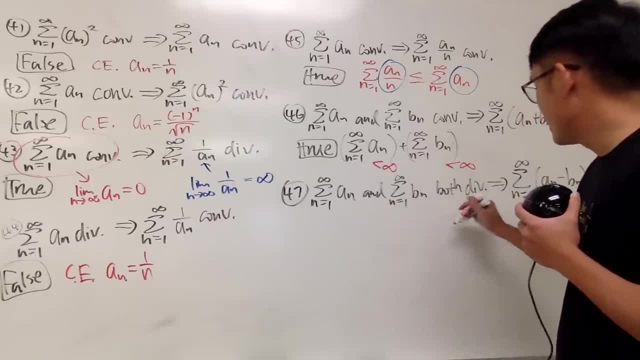 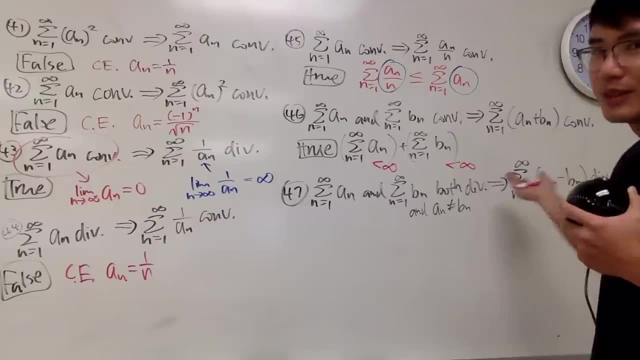 I will also add a little um condition. okay, I will just say: and a n it's not the same as b? n, Otherwise you can just put that 1 over n and 1 over n, and then you get 0,. 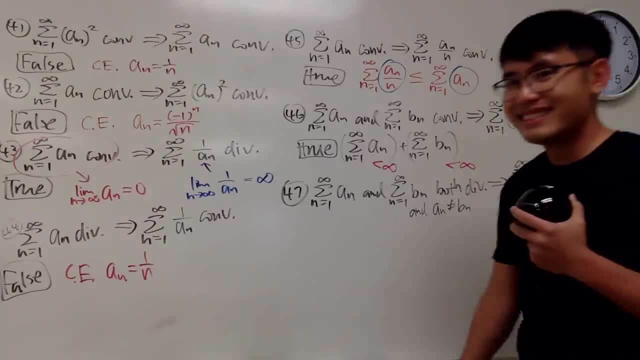 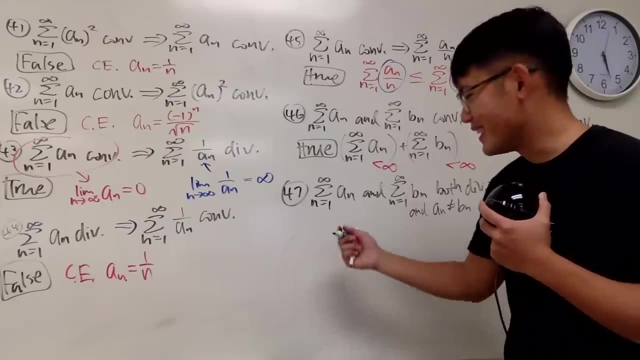 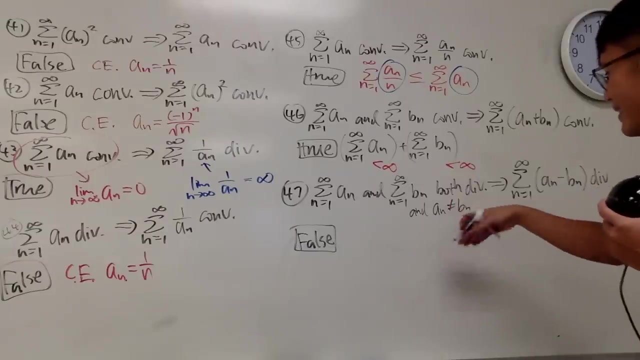 but like no, no, no, Alright, this right here is false. Oops, wrong column, This right here is false, alright, So I'll just put down false. So here is an example, and okay, right here. 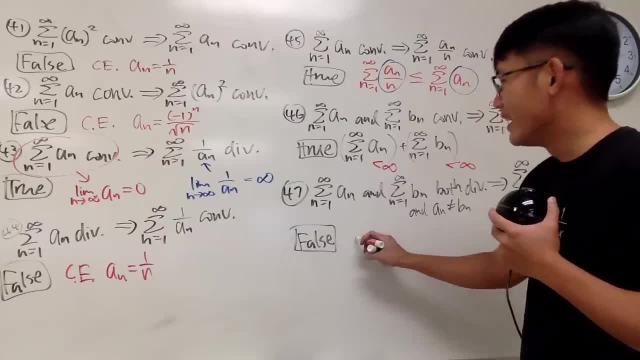 I want a n and b n to not equal to each other for o n, but I can do the following. I can say: uh, count the example. alright, I can take a n to be 1 over n and 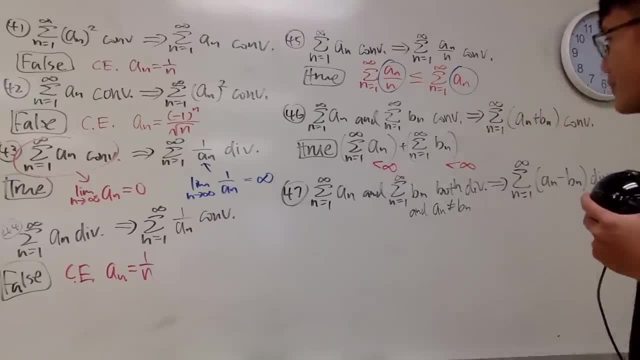 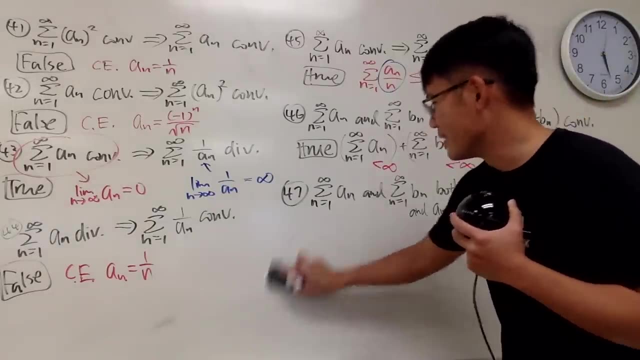 and then you get 0. But like: no, No, No, All right. This right here is false. Oops, Wrong column. This right here is false right, So I'll just put down false. So here is an example. 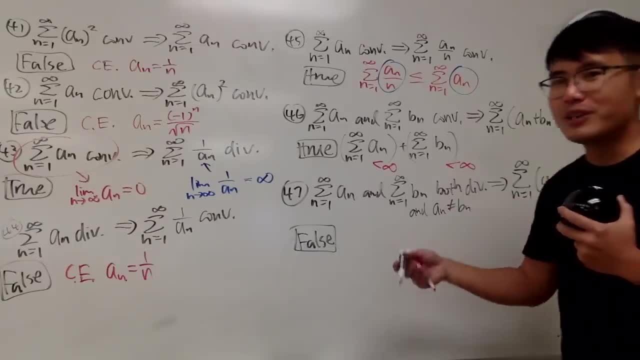 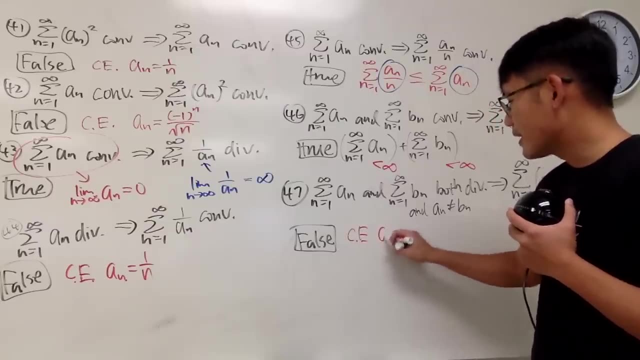 And of course, right here I want a? n and b? n to not equal to each other for o? n. But I can do the following. I can say counter example: right, I can take a? n to be 1 over n and let's say b? n to be 1 over n plus 1.. 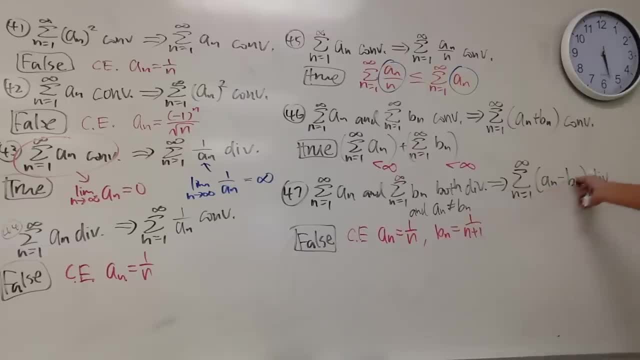 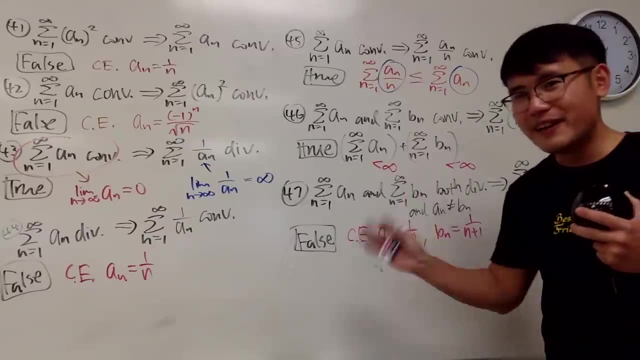 What's this? If you put 1 over n right here, and then minus 1 over b, 1 over n plus 1, you get a telescoping series. So you actually end up with a very nice convergence. And of course, when you subtract, 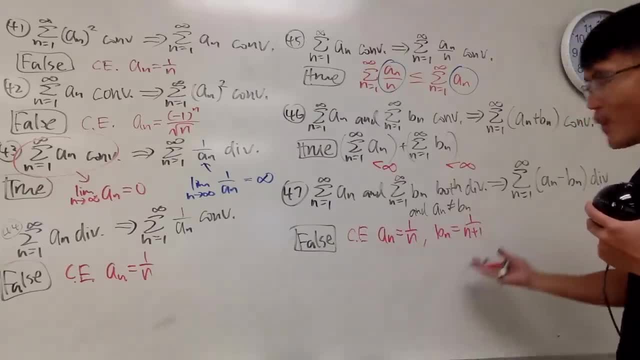 let's say b n to be 1 over n plus 1.. What's this? If you put 1 over n, right here, and then minus 1 over b, 1 over n plus 1, you get a telescoping series. 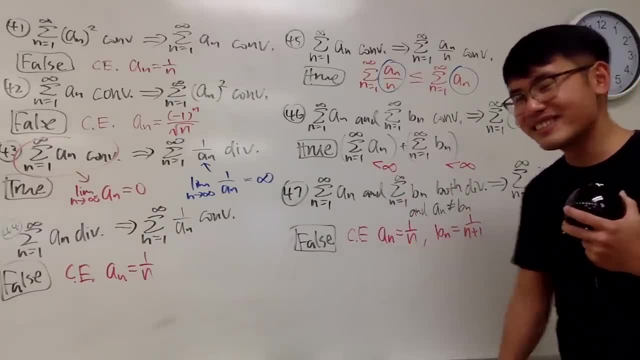 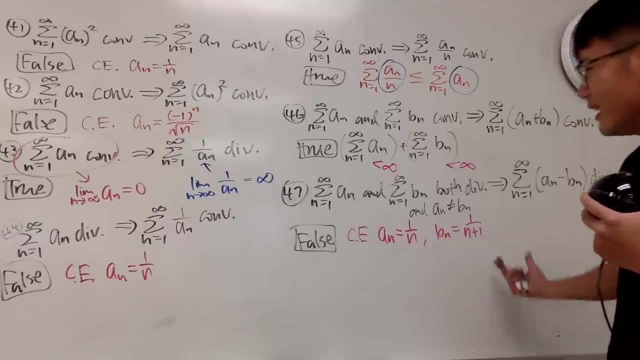 So you actually end up with a very nice convergence. And, of course, when you subtract, you can also, you know, just get the common denominator and you'll see that you can actually get a really nice, uh, convergence. 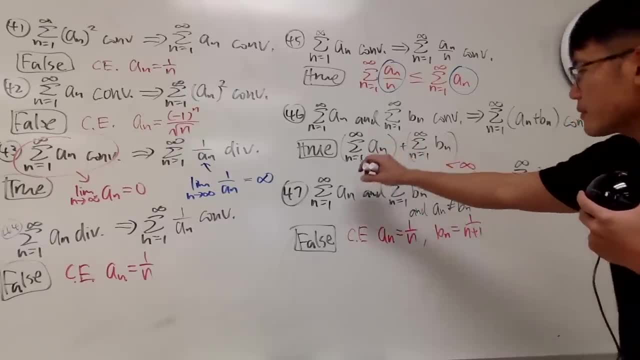 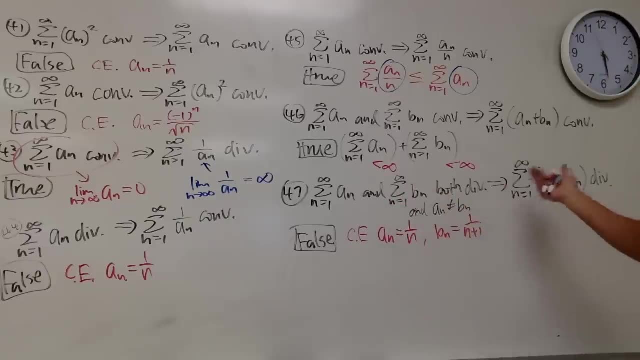 So if both of them diverge, the difference of two divergent doesn't have to be divergent all the time. Of course, this can be still true, but it's not um true all the time. so this is: 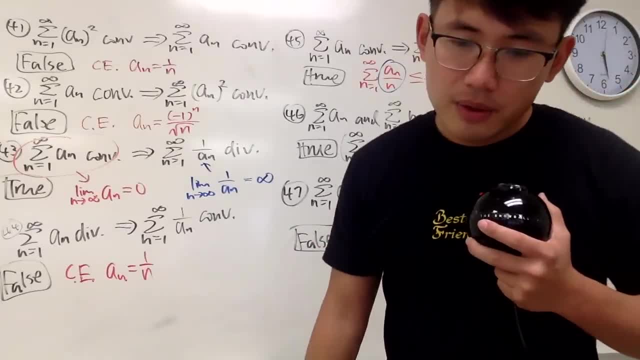 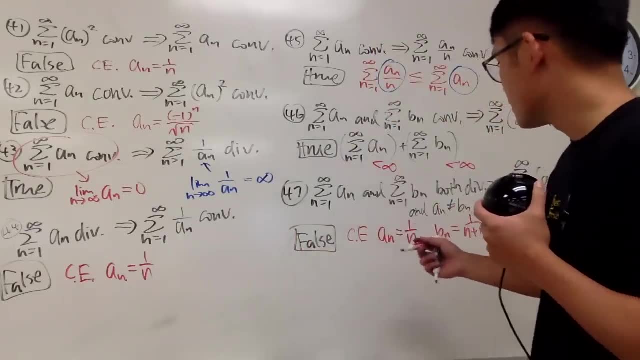 uh, false implication all the time right. So that's it Alright. now a n, b n the series for that both diverge, let's see. So I'll write this down again. number 48.. 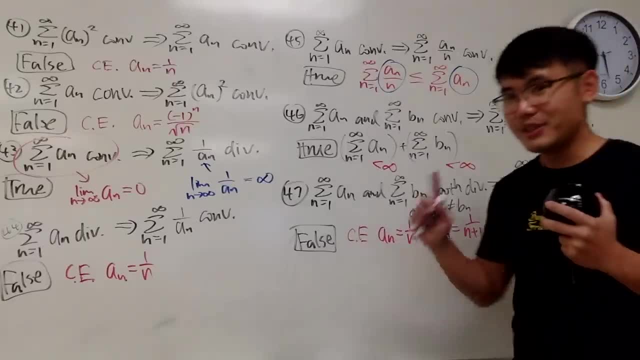 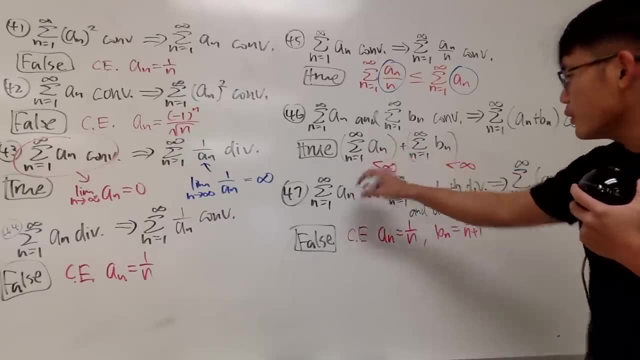 you can also just get the common denominator and you'll see that you can actually get a really nice convergence. So if both of them diverge, the difference, the difference of two divergent, doesn't have to be divergent all the time. Of course this can be still true. 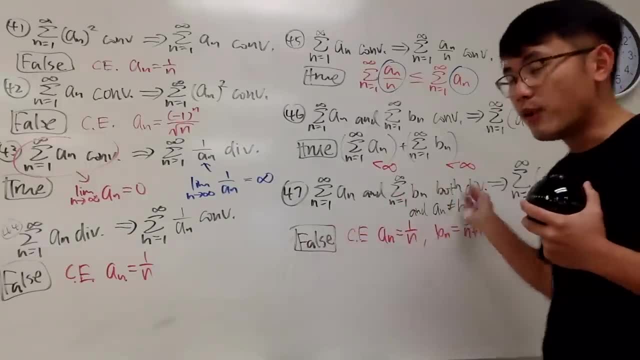 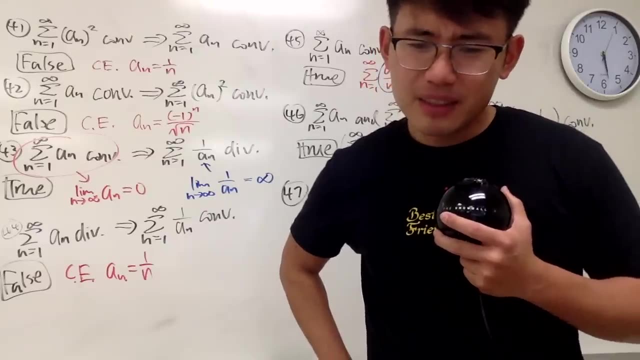 but it's not true all the time, So this is a false implication. all the time, right. So that's it All. right Now a n b? n the series for that both diverge, Let's see. So I'll write this down again. 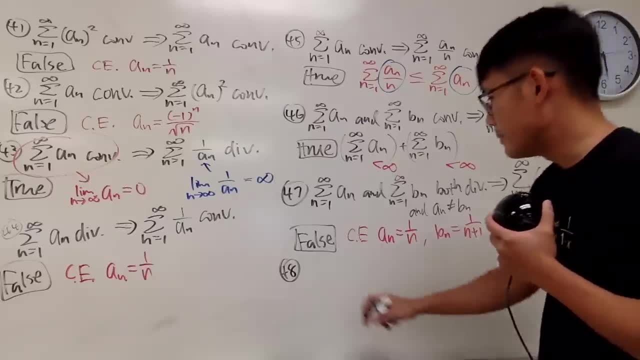 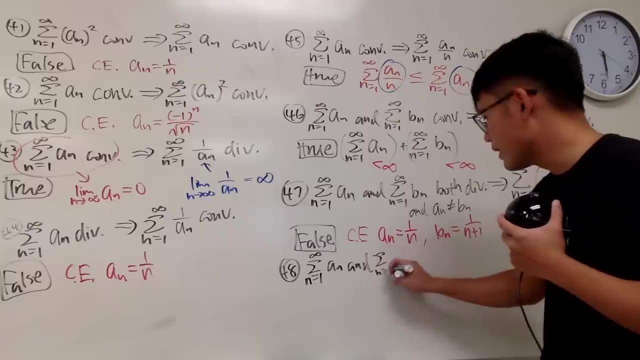 Number 48.. I think I should change the marker. Maybe let me get up to 50.. The sum of n goes from 1 to infinity a n and the sum of n goes from 1 to infinity b n. both diverges. 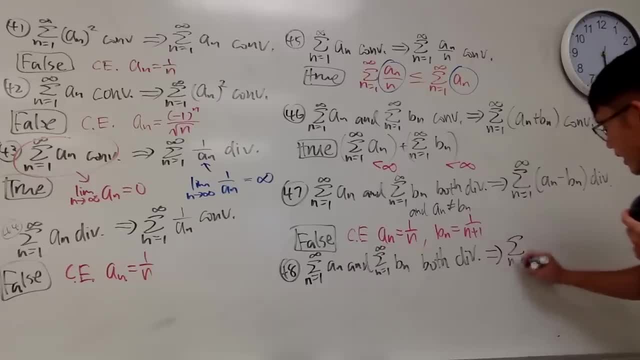 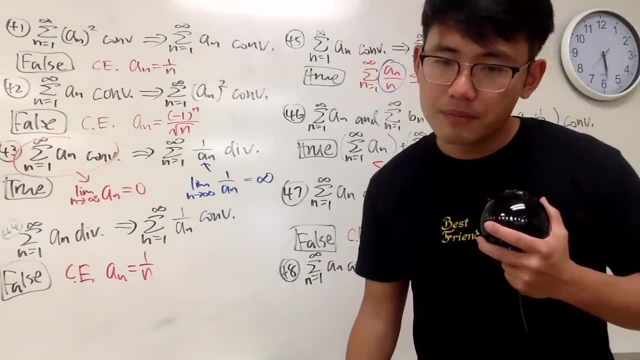 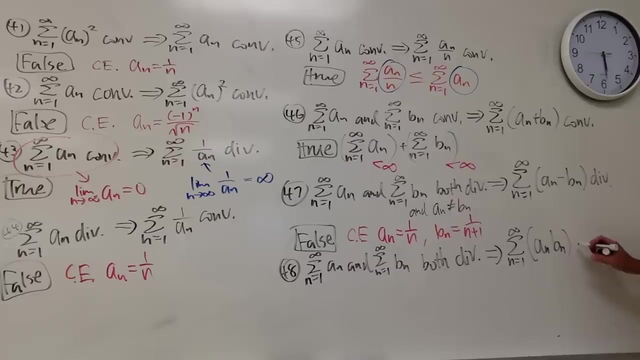 Both diverge. Well, what if we look at the product of a, n, b, n like this: Is it possible that, okay, it's that if this diverges, that diverges, and when you multiply that, hmm, this right here must diverge. 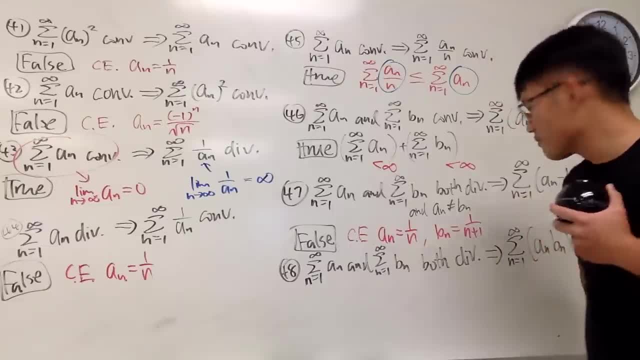 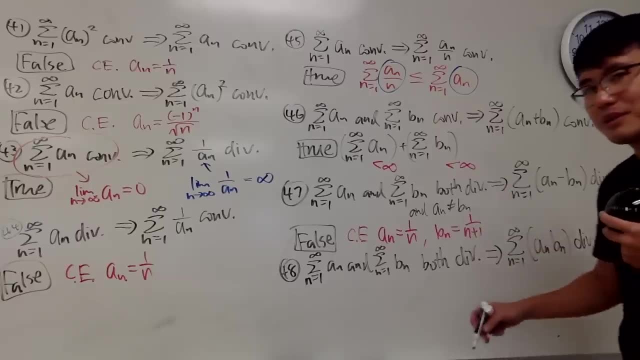 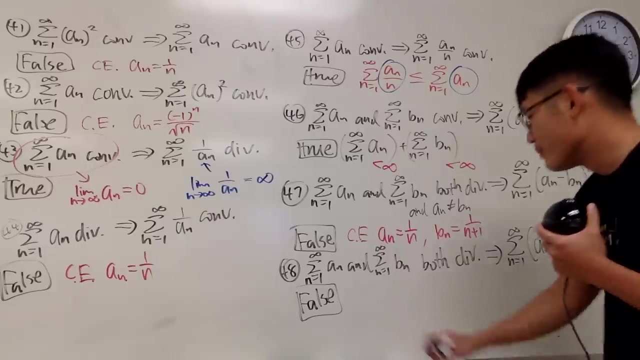 So is it possible to end up with a convergent? What do you guys think? Of course, we can also have this little condition, but this right here is, of course, false. Why? Because counter example. What's a prime example of a divergent? 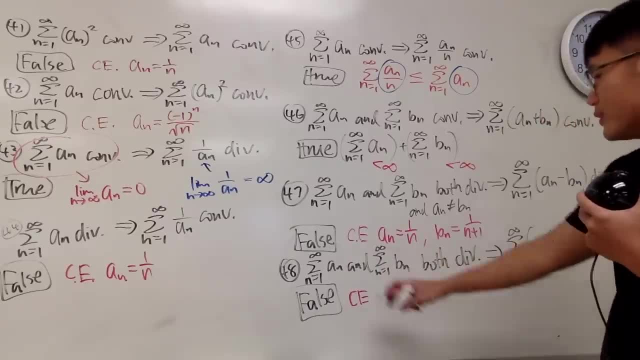 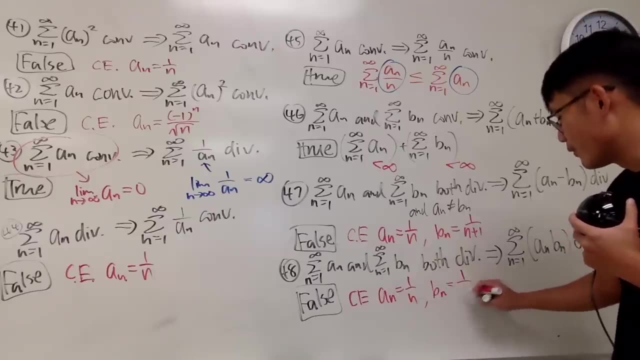 Of course, you can just do the harmonic series right, So you can just do this. You can do this right here, which is: a? n equals 1 over n, And if you don't want b? n to be the same, what you can do is just do 1 over square root of n. 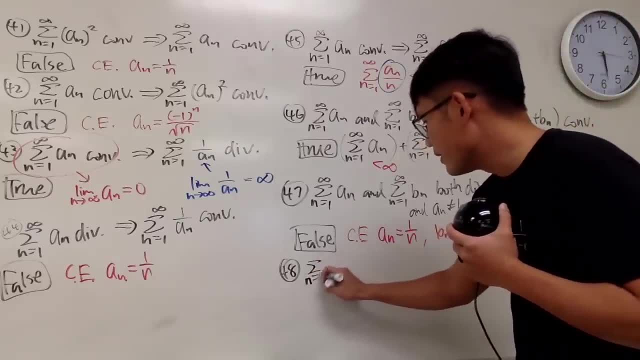 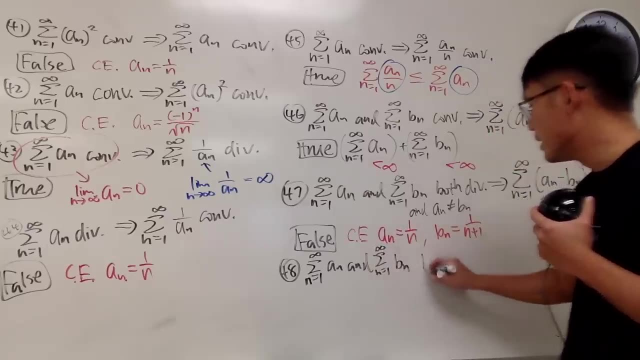 I think I should change the marker. maybe let me get up to 50.. The sum of n goes from 1 to infinity a- n and the sum of n goes from 1 to infinity b- n. both diverges. 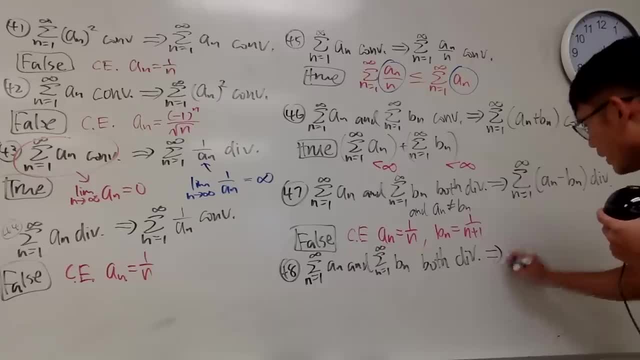 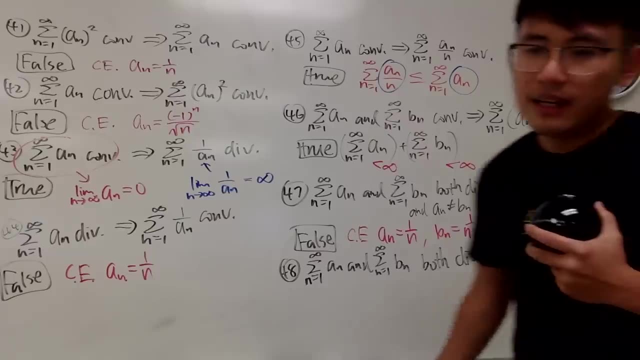 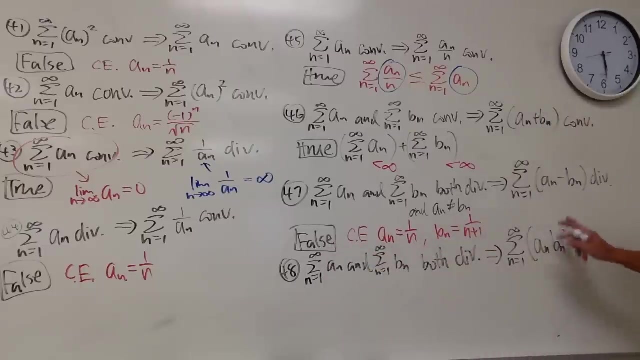 both diverge. Well, what if we look at the product of a, n, b, n like this: Is it possible that, okay, it's that if this diverges, that diverges. and when you multiply that, um, hmm, 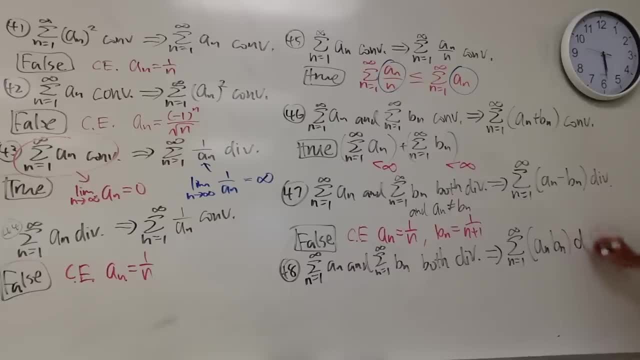 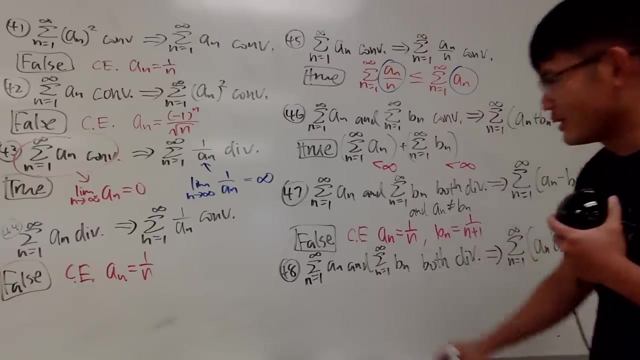 this right here must diverge. So is it possible to end up with a convergent? What do you guys think? Of course we can also have this little condition, but this right here, it's of course false. Why? 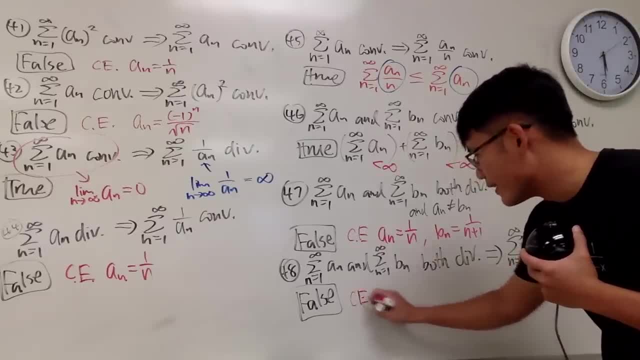 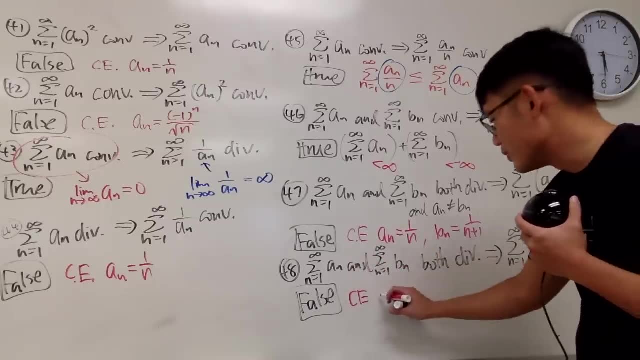 Because counter example, What's a prime example of a divergent? Of course you can just do the harmonic series right. So you can just do this right here, which is: a n equals 1 over n, and if you don't want b n to be the same, 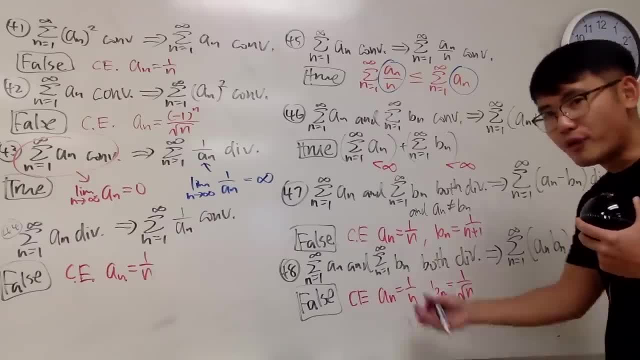 what you can do is just do 1 over square root of n. Both of them diverge. but look at this right. here We're not saying the series of a? n times the series of b? n. We're talking about the series of a? n. 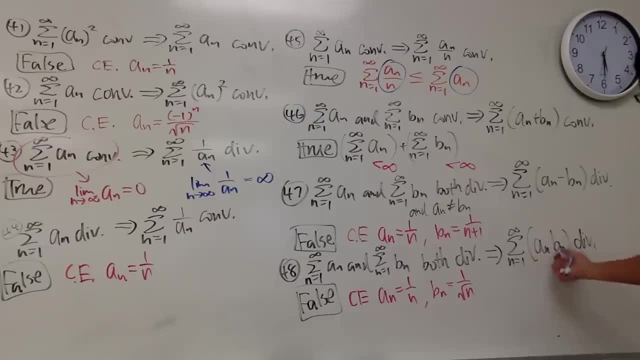 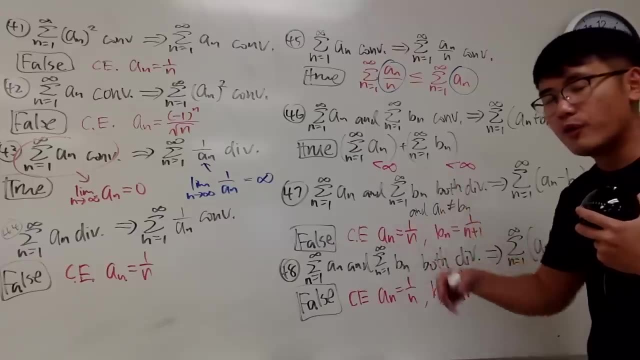 b, n multiplying together first. So if you do this, you do 1 over n times 1 over square root of n, which you end up with 1 over 3 to the 1 over n to the 3 half power. 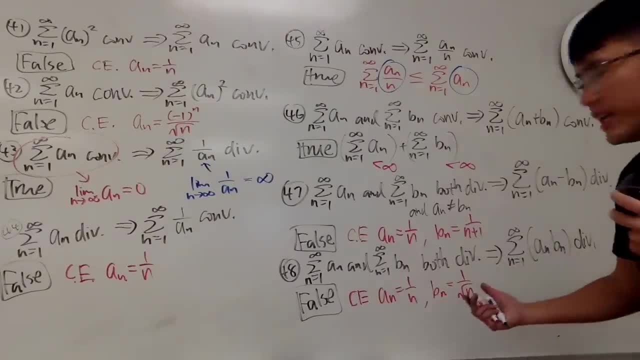 Both of them diverge. But look at this right here We're not saying the series of a? n times the series of b? n. We're talking about the series of a n b? n multiplying together first. So if you do this, 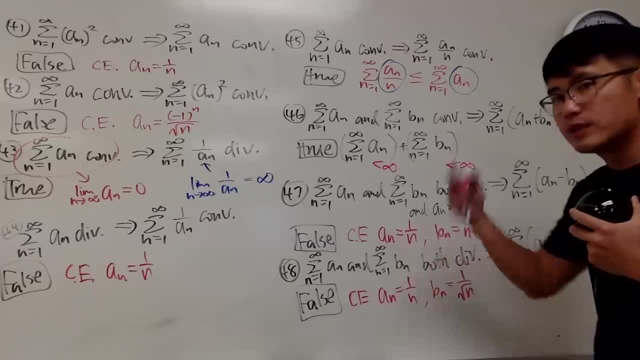 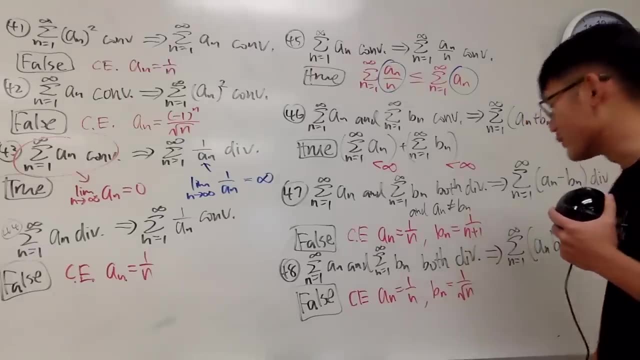 you do 1 over n times 1 over square root of n, which you end up with 1 over n to the 3 half power and you get a p series That's actually convergent. So this right here would be a counter example. 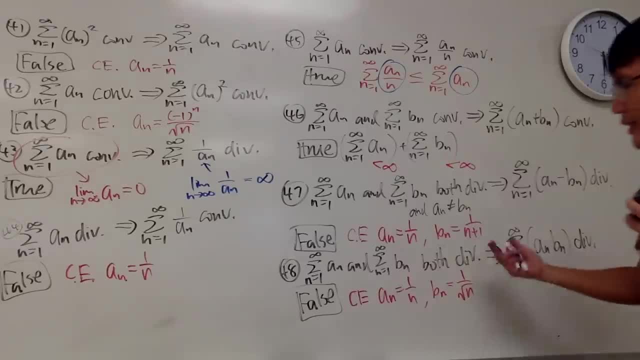 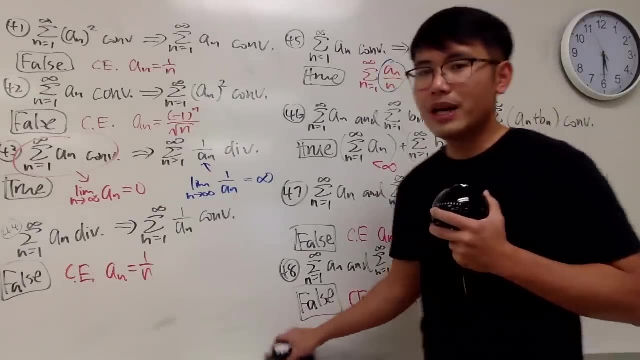 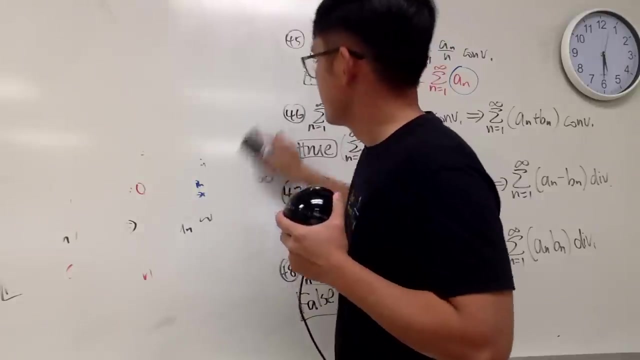 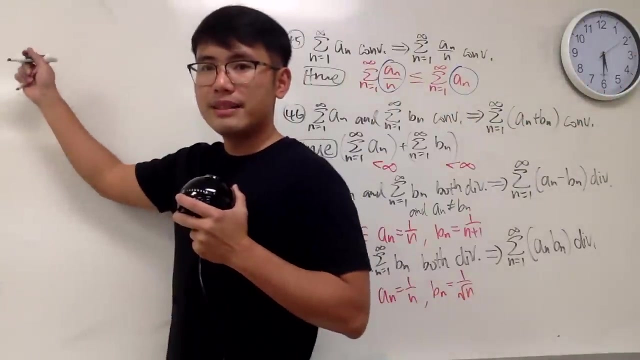 and you get a p series. that's actually, that's actually convergent. So this right here would be a counter example for this little statement. So, okay, now we are going to move on to number 49.. Alright, number 49. 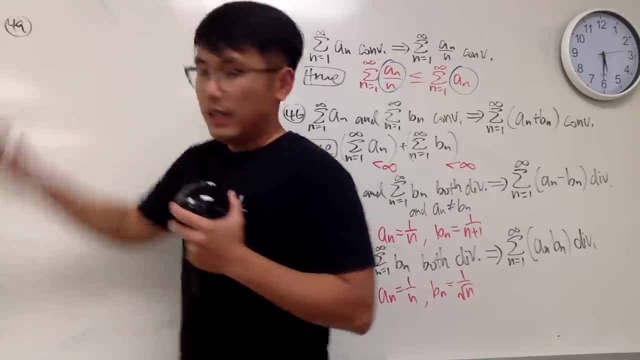 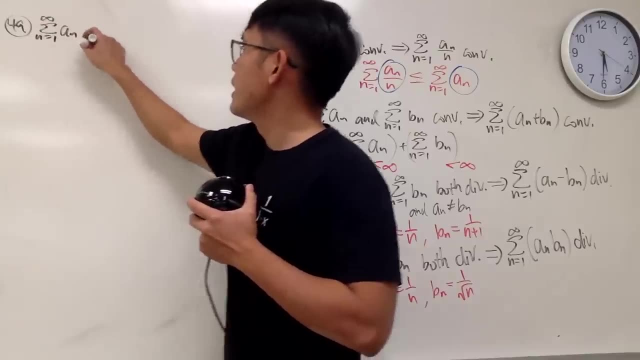 right here. Okay, So 49.. Uh, okay, if the series of a, n, b, n. let's see if the series 1 to infinity, a, n and the series b n. this time I want them to be both. 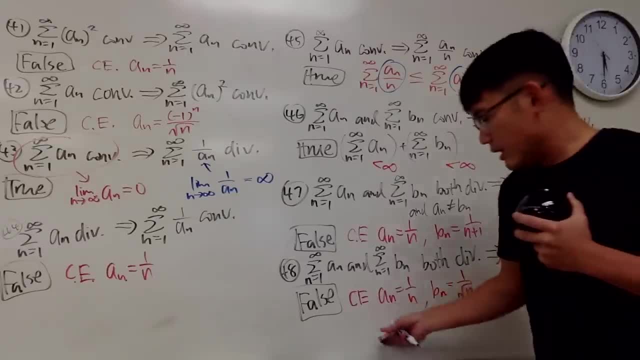 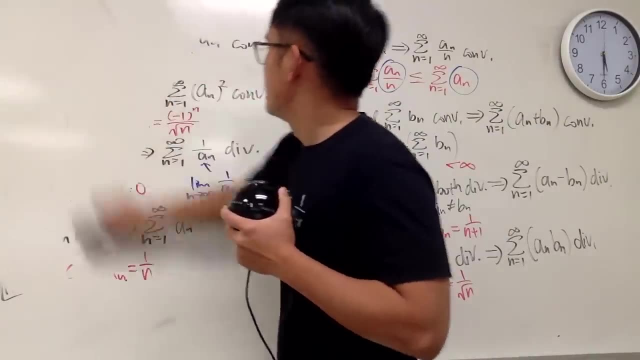 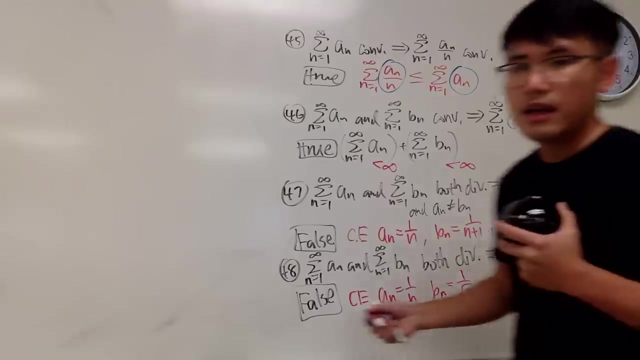 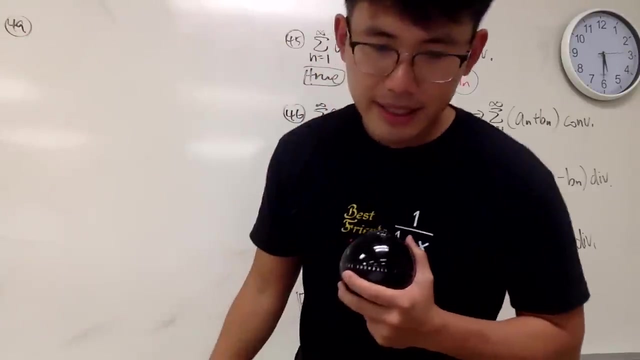 for this little statement. So that's good. OK, Now we are going to move on to number 49.. All right, Number 49, right here. OK, So 49.. OK, So we have a series of a, n, b, n. 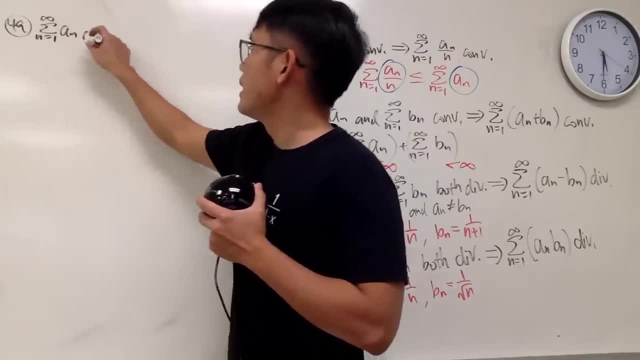 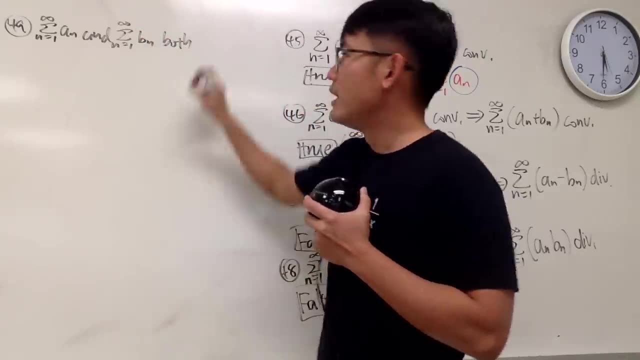 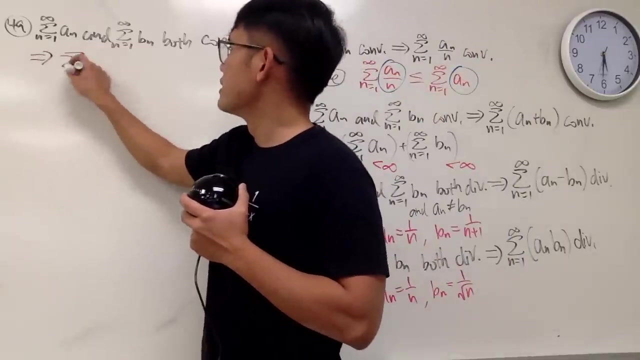 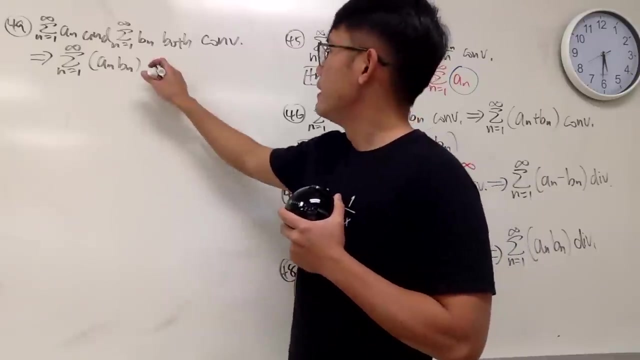 Let's see: We have the series 1 to infinity a, n and the series n equals 1 to infinity b, n. This time I want them to be both convergent. Then do we must get the sum as n equals 1 to infinity, parentheses a, n, b, n. 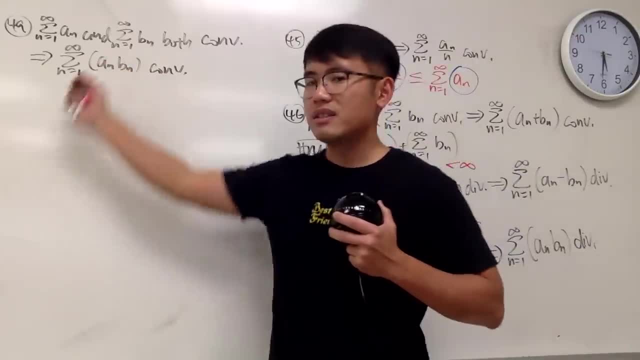 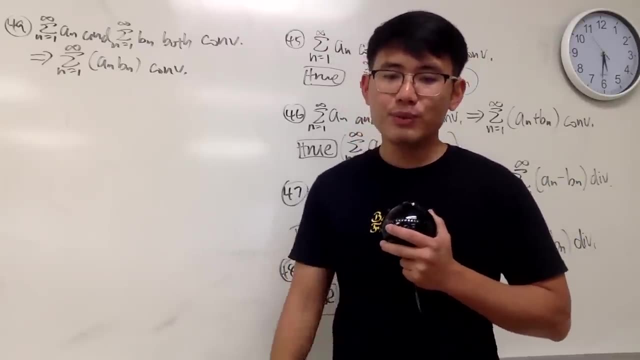 Do we get a convergent sum? Let's see. So we have a series of a, n, b, n inside. if you multiply first, And of course, if you want to make this a little more challenging, you can just say: a n, b, n are not the same. 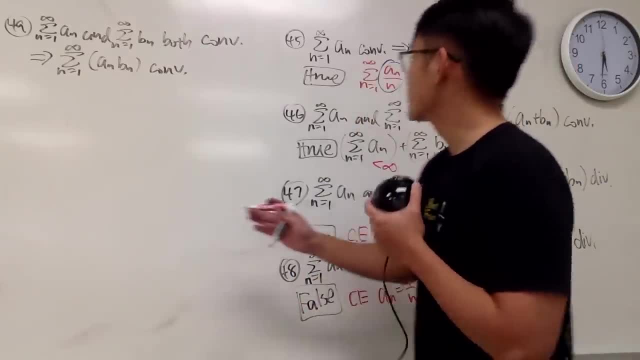 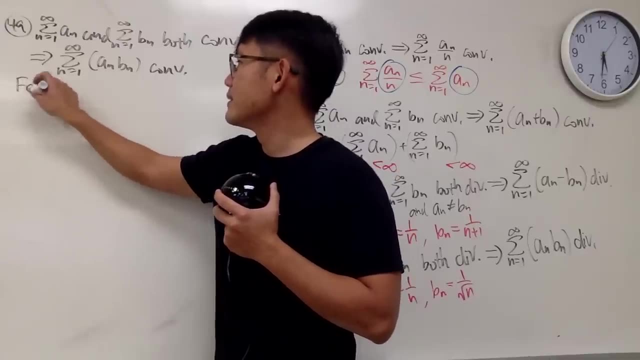 But it doesn't really matter in this case. Anyway, this is actually really similar to one of the questions that I just erased. I just realized that, But this right here is again false. Let me give you an example for this. 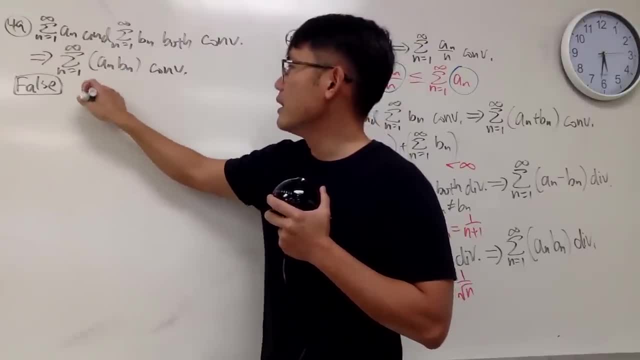 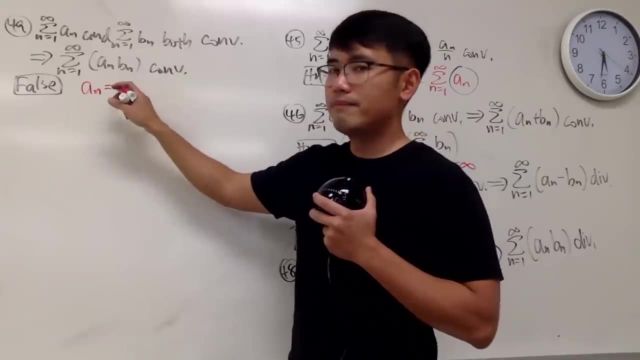 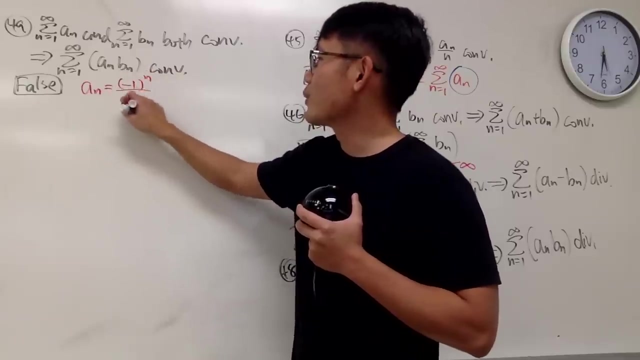 Well, I can just say that a n, the a n equal to. I need to make sure that a n, the series of a n, actually converge. I will do an alternating series. Let's do a negative. 1 raised to the nth power over square root of n. 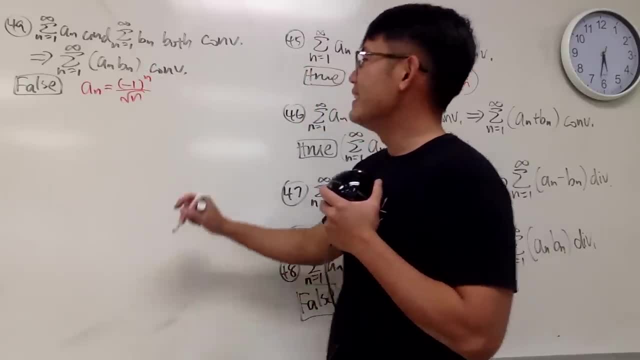 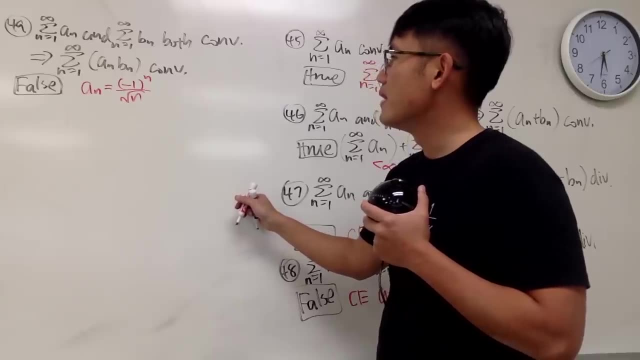 How's that Good? huh, And I will do the other one. Let's see. OK, So for b? n, let's do this. Negative 1 to the nth: power over. I will also do the same kind of thing. 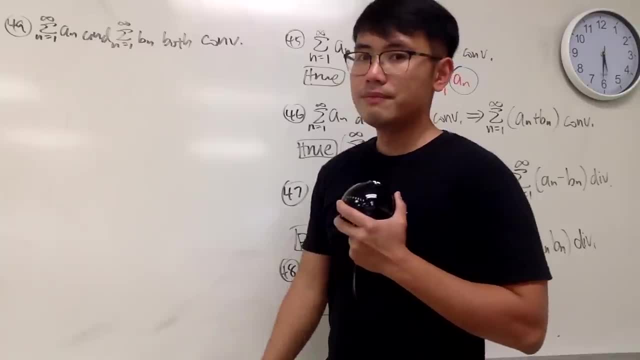 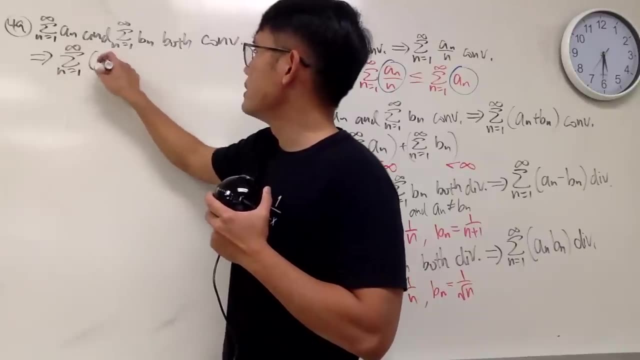 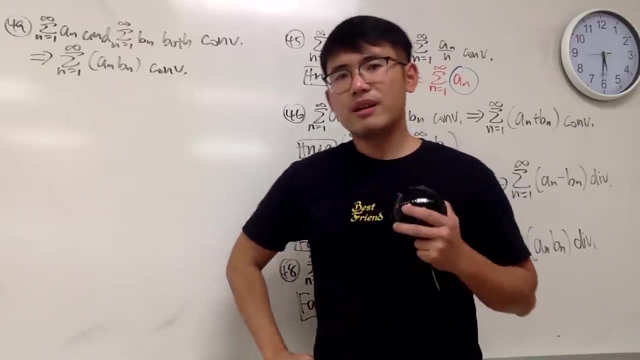 convergent, Then do we must get the sum as n goes from 1 to infinity parentheses- a, n, b, n, Hmm. Do we get a convergent a n, b, n inside if they multiply first? Hmm, And of course, if you want, 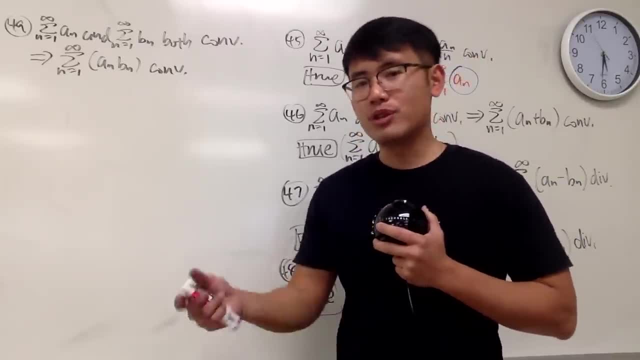 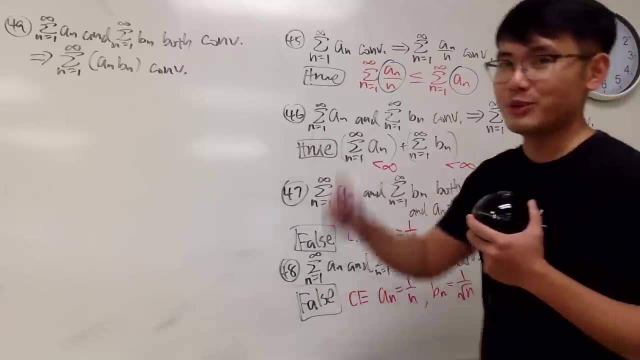 to make this slightly more challenging, you can just say: a, n, b, n are not the same, but uh, it doesn't really matter in this case. Anyway, this is actually really similar to one of the questions that I just erased. I just realized that. 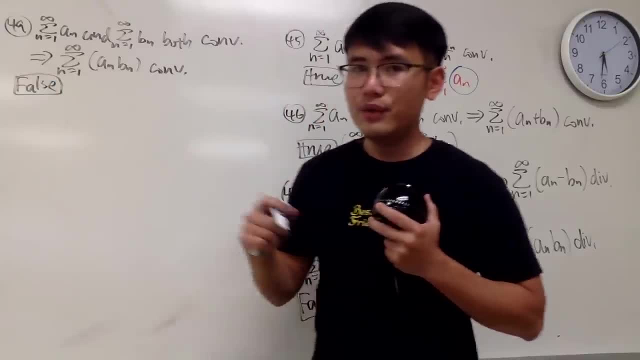 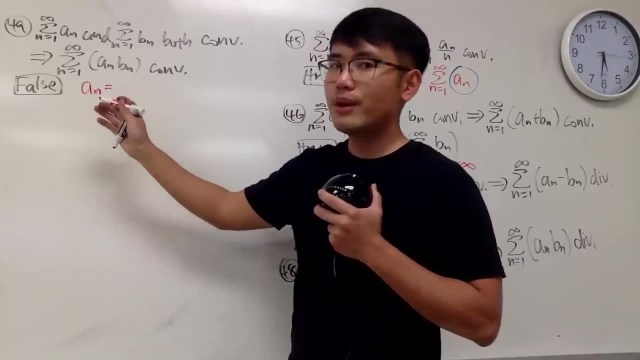 But this right here is again false. Let me give you an example for this. Well, I can just say that a n, that a n equal to, I need to make sure that a n, the series of a n, actually converge. 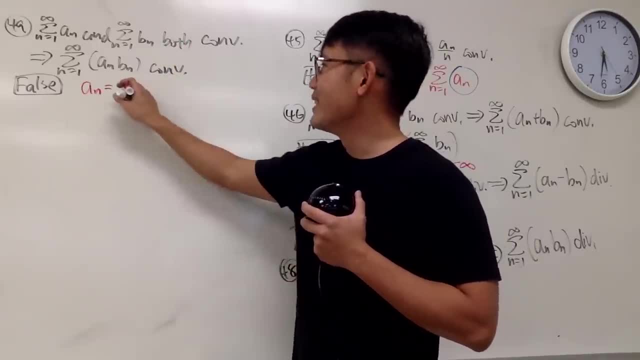 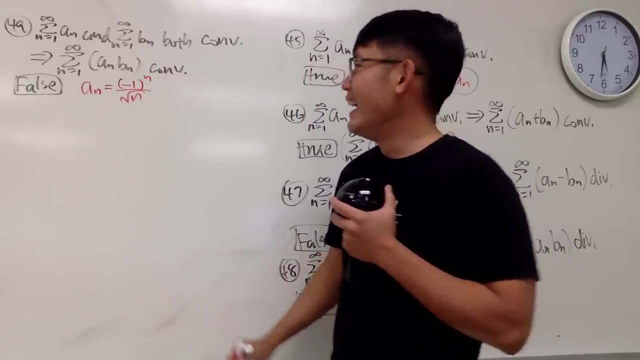 But I will do an alternating series. Let's do a negative one, raised to the nth power over square root of n- How's that Good huh? And I will do the other one. Let's see, Okay, So. 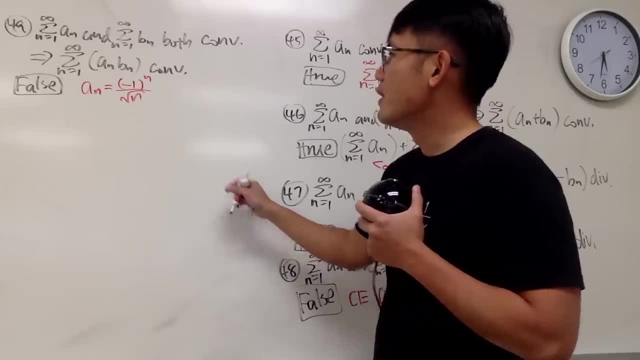 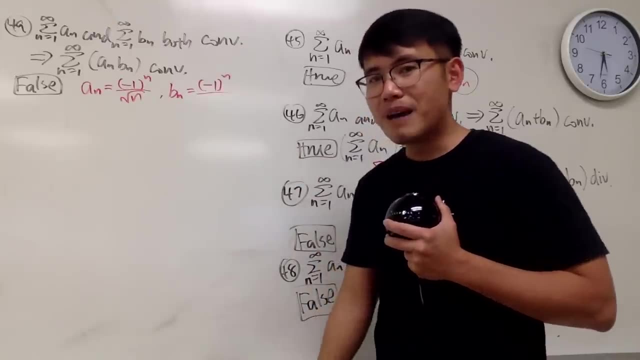 for b? n. let's do this Negative one to the nth power over. I will also do the same kind of thing, But if you don't want a n- b n to be the same, then this is what you can do. 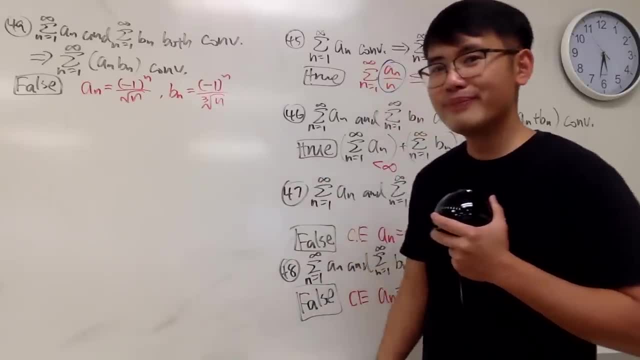 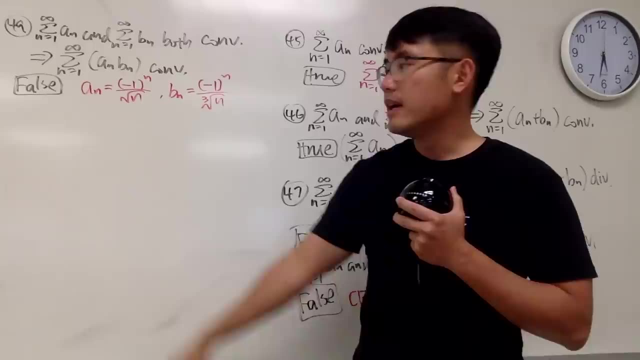 You can just do the cube root of n. Now here's the deal: When you multiply them, negative one to the nth power times, negative one to the nth power, is just always going to be one Square root of n, which is n to the one-half power. 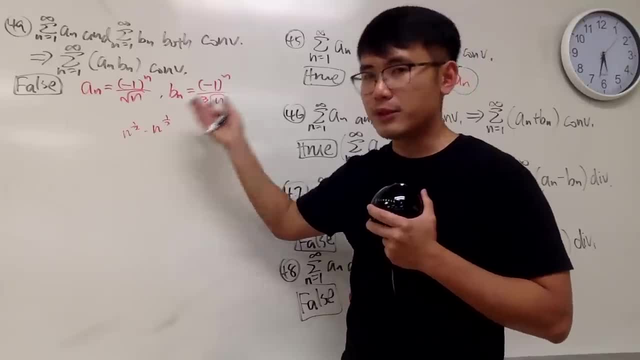 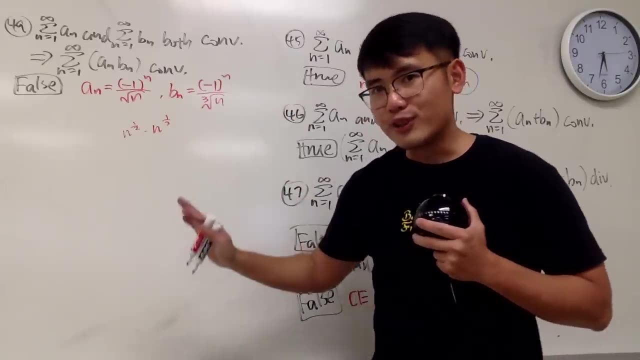 times n to the one-third power you can just add It's going to be less than one. Right n to a power that's less than one, That's like five over six. That's a divergent. So this right here. 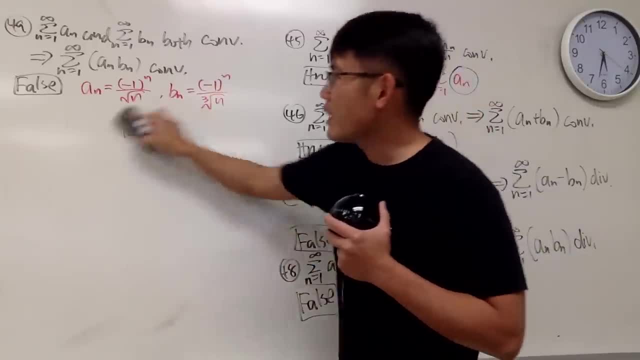 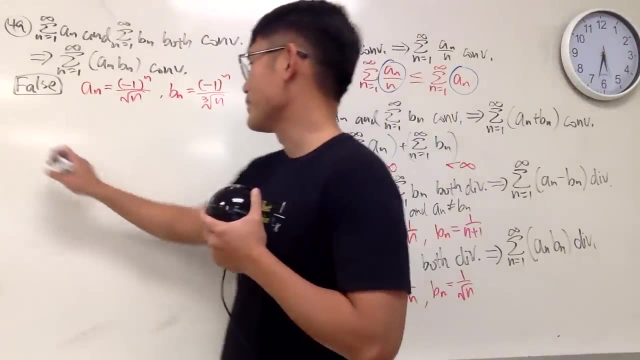 it's false. It's possible to end up with a divergent right here in this case. So hopefully it gets all like these true-false questions Right Now. just to kind of take a little break right here, let's take a look. 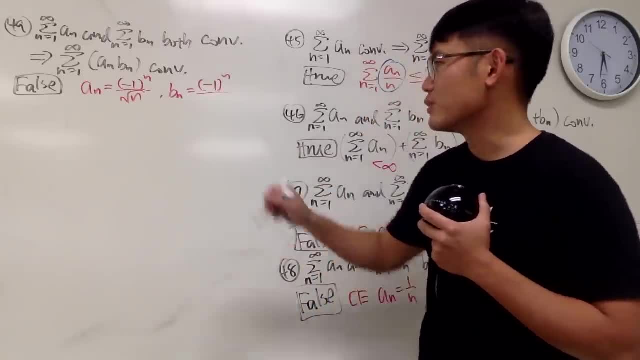 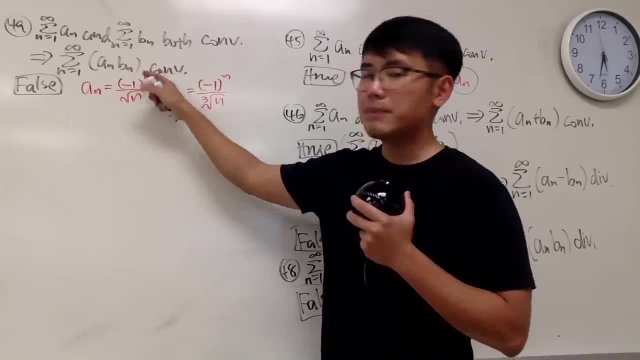 But if you don't want a, n, b, n to be the same, then this is what you can do. You can just do the cube root of n. Now here's the deal. When you multiply them, negative 1 to the nth power times negative 1 to the nth power. 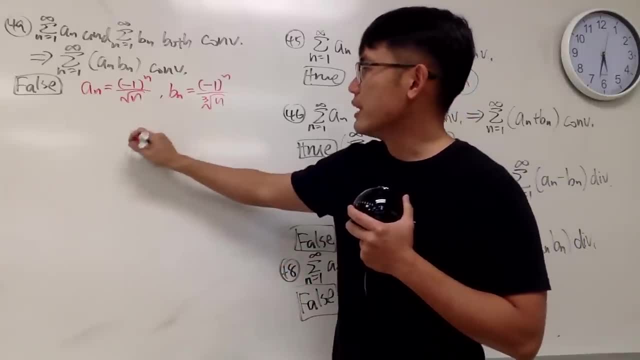 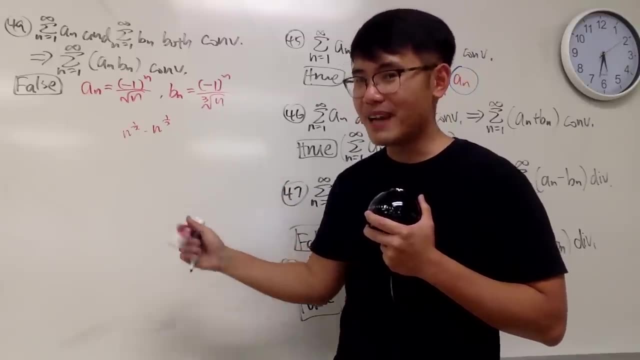 is just always going to be 1.. Square root of n, which is n to the 1 half power, times n to the 1 third power, you can just add: It's going to be less than 1, right n to the 1 half power. 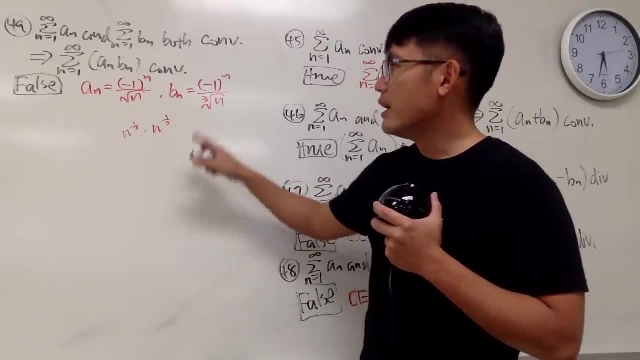 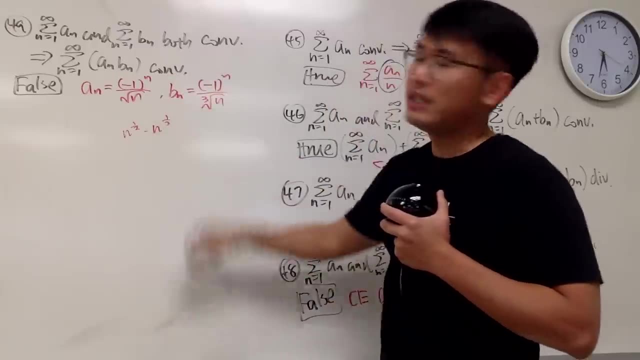 And n to the power, that's less than 1, that's like 5 over 6.. That's a divergent. So this right here is false. It's possible to end up with a divergent right here with these examples. So hopefully you guys all like these true-false questions, right. 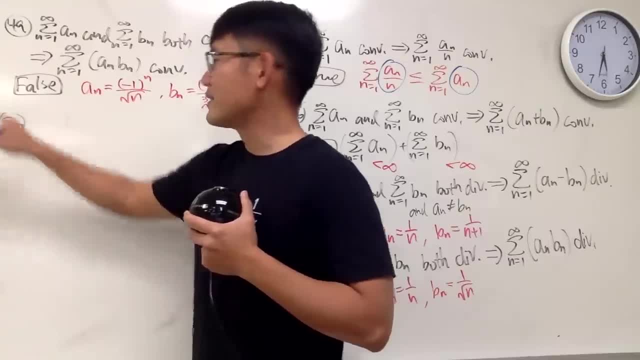 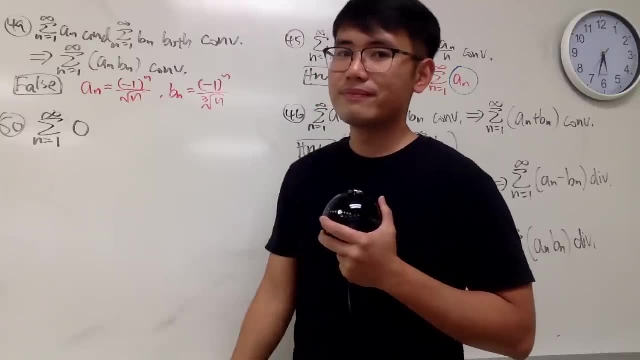 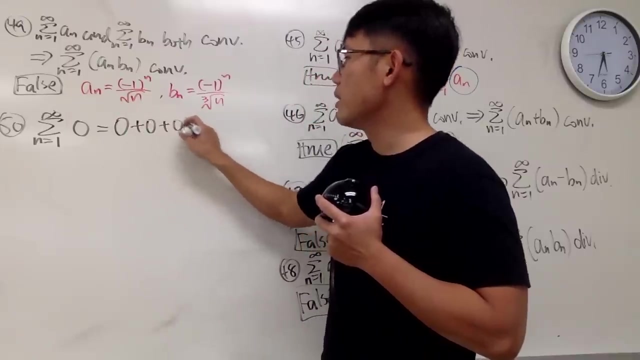 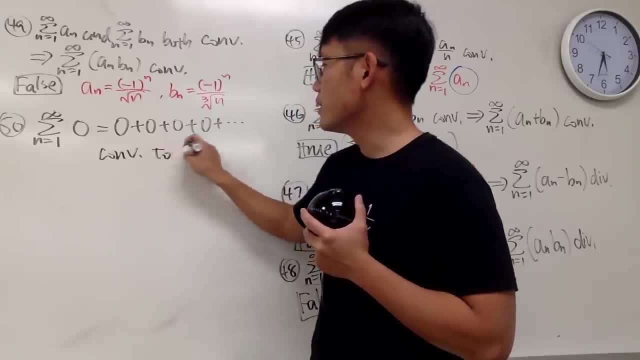 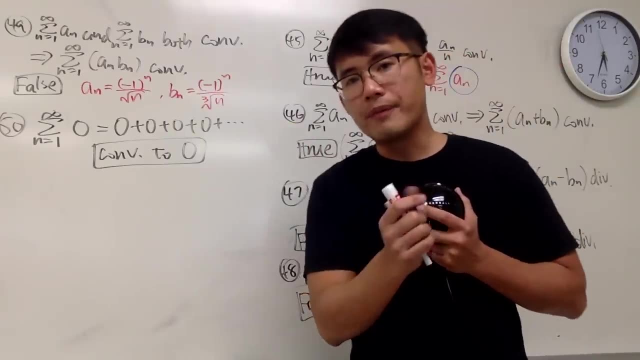 This right here converges to 0.. Why, Again, all these 0s that are solid 0s? it's not like 0.0001, right? This 0 is not from the limit of any kind, It's just a number. 0. 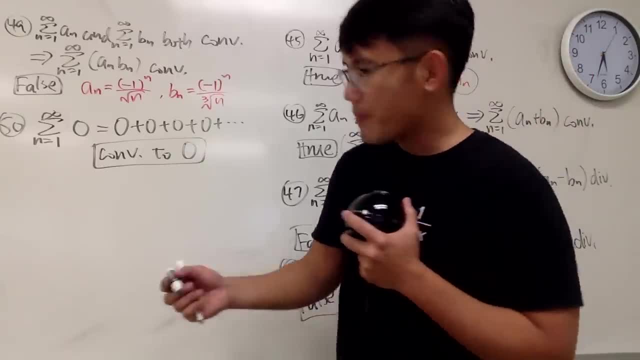 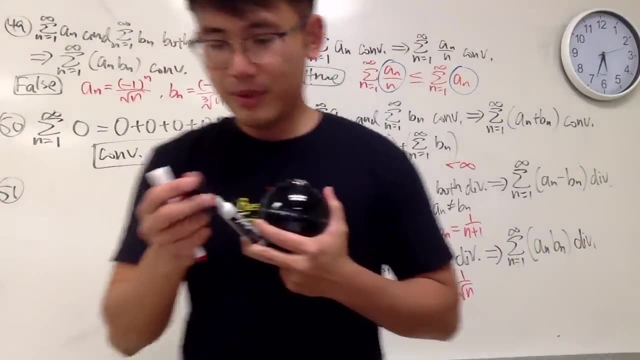 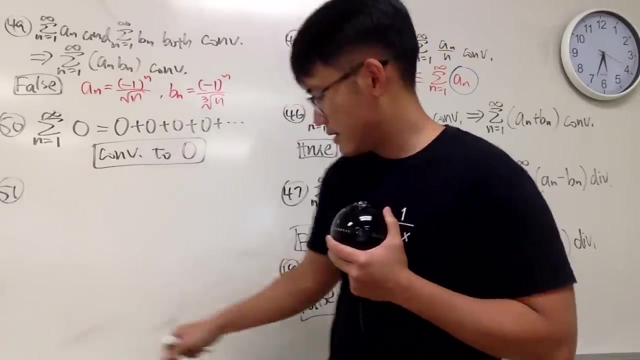 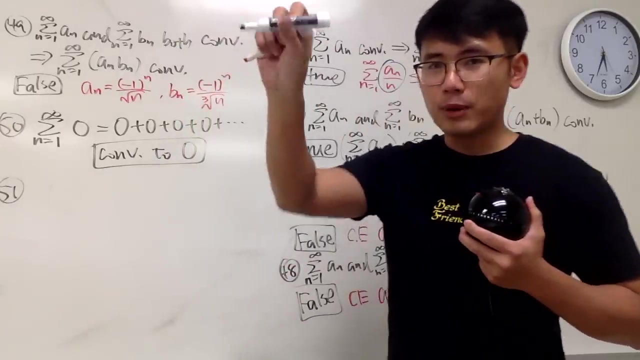 So that's all Very, very nice. Now number 51.. I am going to change the marker. All right, I'm going to change the marker. I have another one: X-pole marker for the wing. seriously, X-pole marker for the wing. 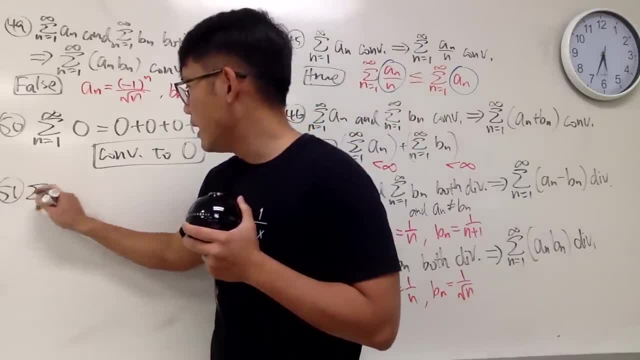 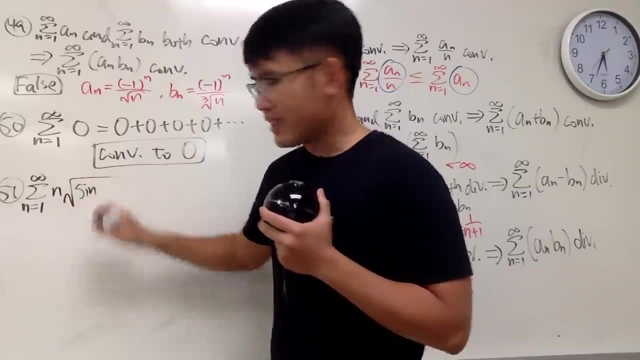 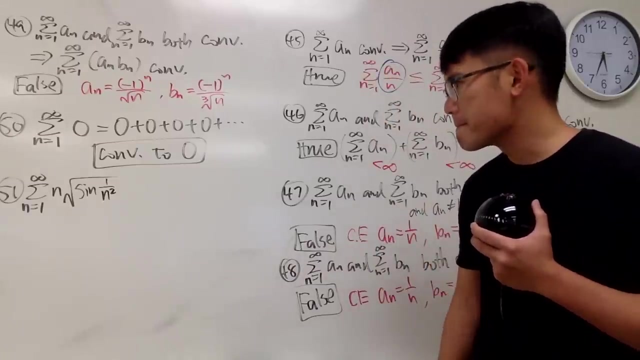 Anyway, number 51.. We are going to look at the sum as n goes from 1 to infinity And here we have n times the square root- Oh my god Sine- of 1 over square. Again, very similar to one of the examples I showed you earlier. 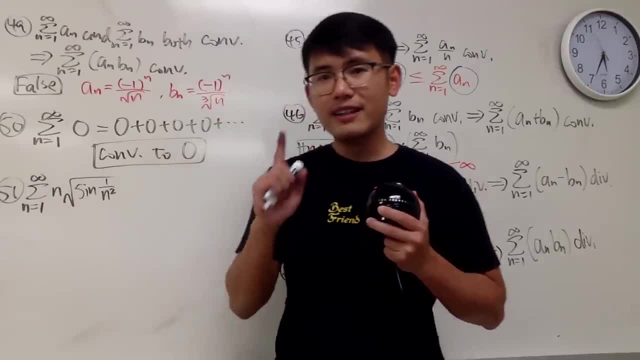 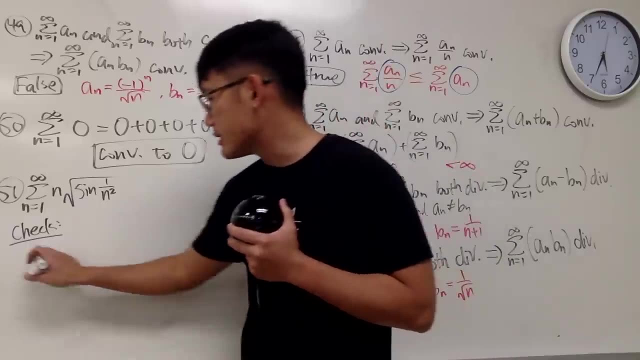 It's infinity times 0 if you take the limits. Let's try the test for divergence first. So right here, let's go ahead and check What if we just take the limit, as n goes to infinity. So we have to put this down. 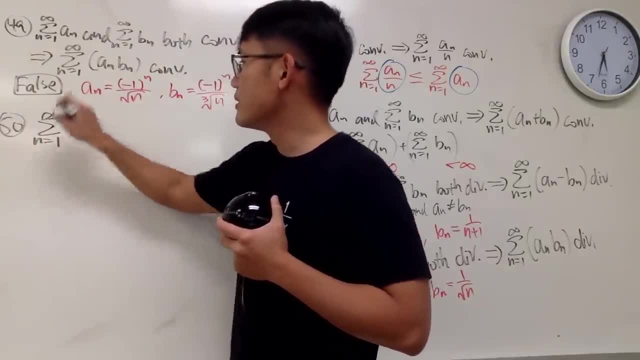 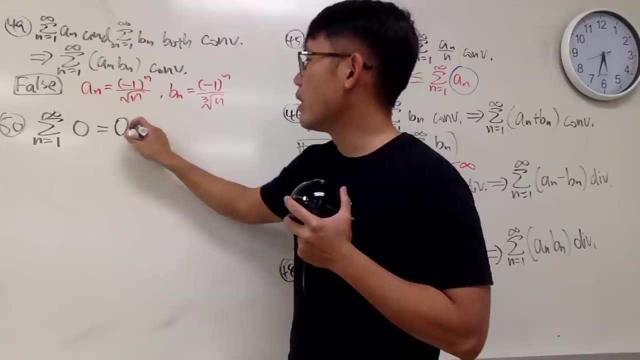 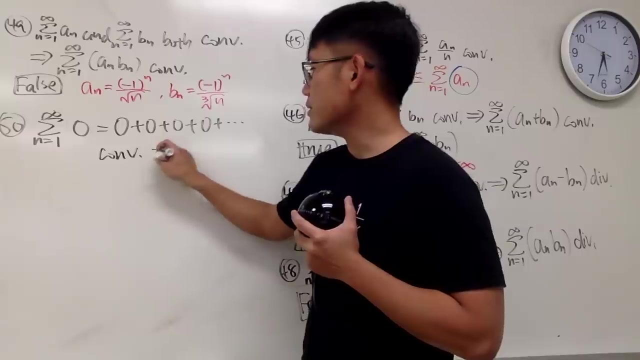 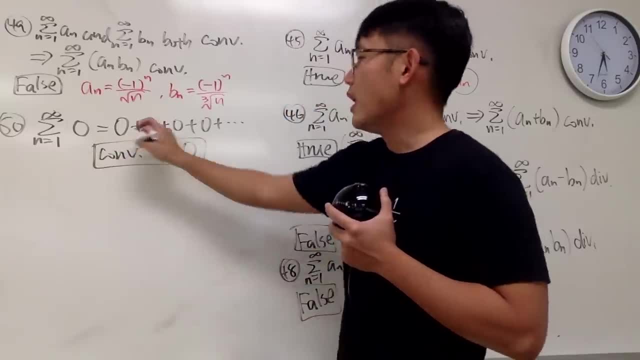 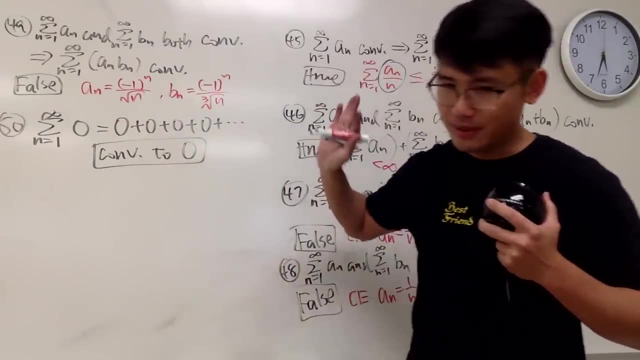 to zero. Why, Again, all these zeros that are solid zeros? it's not like zero point zero, zero, zero, one Right, This zero, it's not from the limit of any kind, It's just number zero. So that's all. 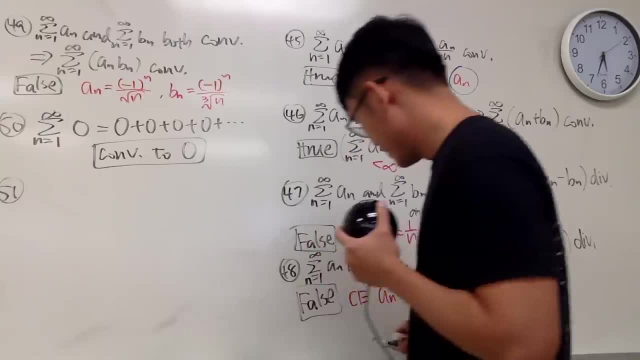 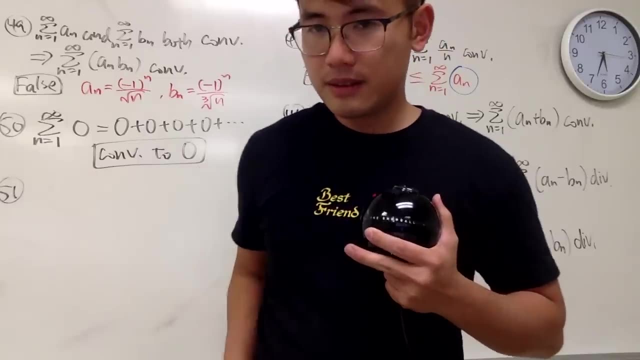 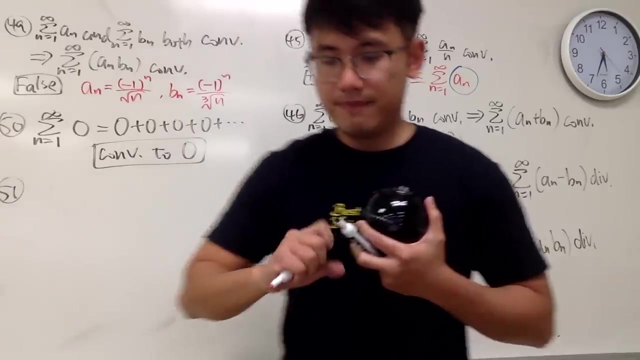 Very, very nice. Now, number fifty-one: I am going to change the marker. Right, I'm going to change the marker. I have another one: X-point marker for the wing. seriously, X-point marker for the wing. Anyway, 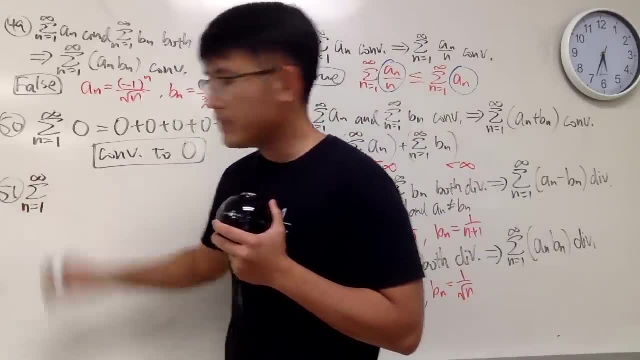 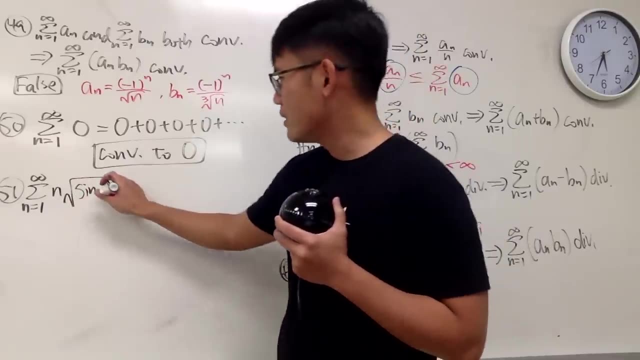 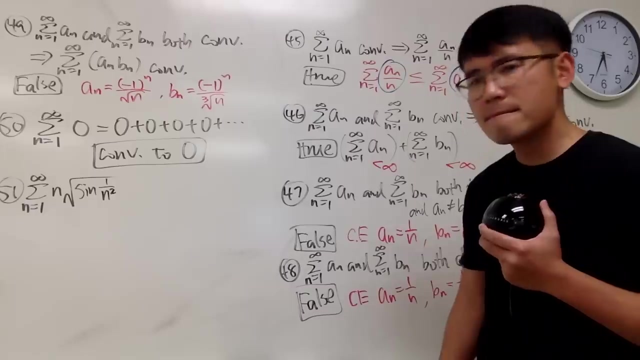 number fifty-one. We are going to look at the sum as n goes from one to infinity, And here we have n times the square root- oh my god, sine of one over square. Again, very similar to one of the examples that we did earlier. 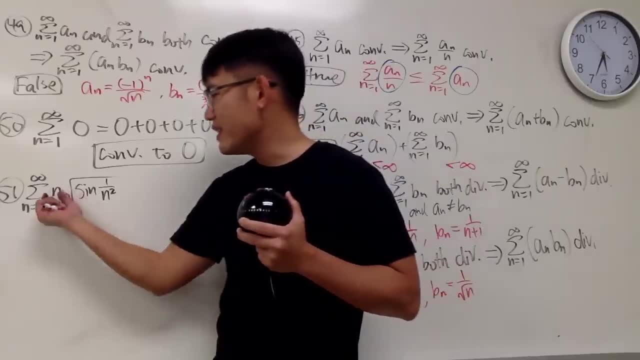 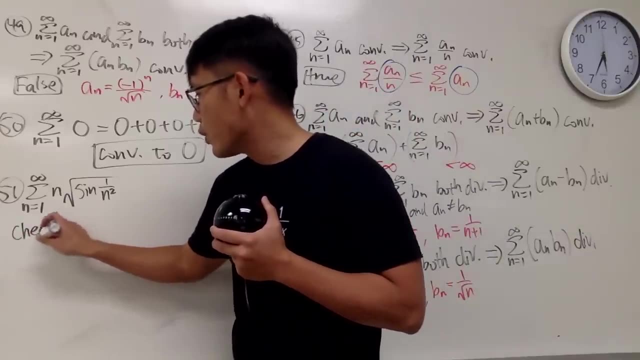 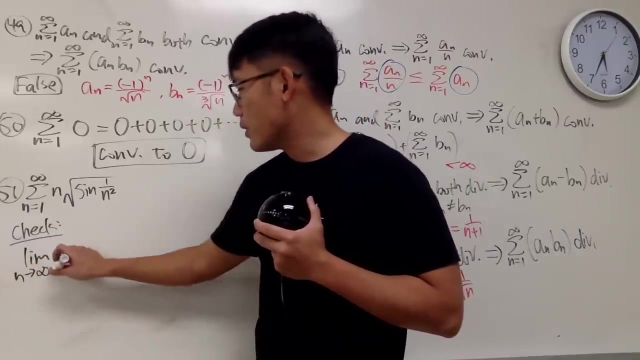 It's infinity times zero if you take the limits. Let's try the test for divergence first. So right here, let's go ahead and check what if we just take the limit, as n goes to infinity. So we have to put this down. 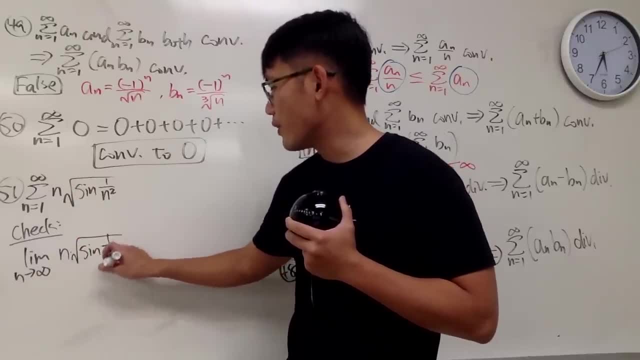 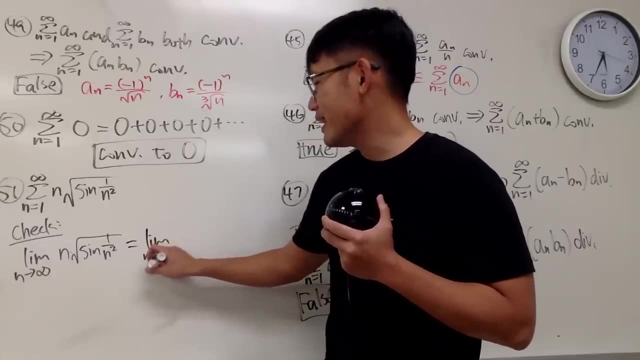 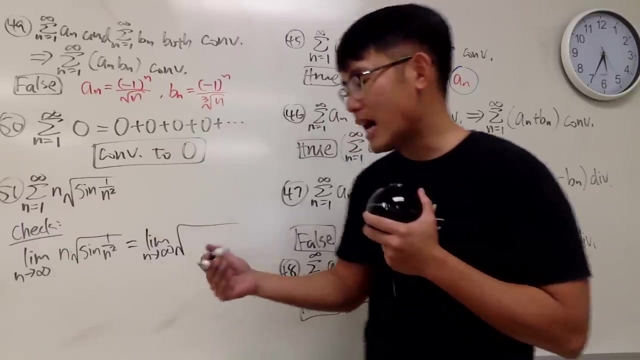 n times the square root of sine of one over n squared. here's the deal. it's not so bad at all. This is n goes to infinity. open the square root because I can actually divide the n inside and it becomes. let me just write this down: 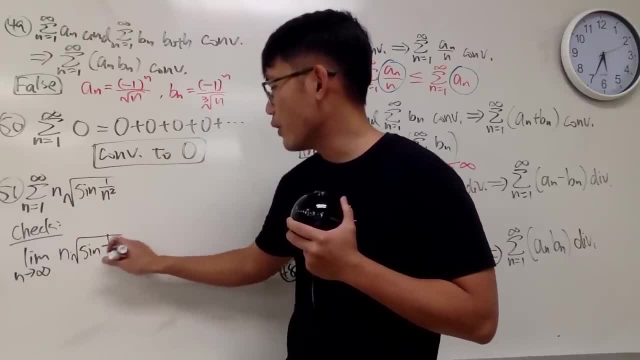 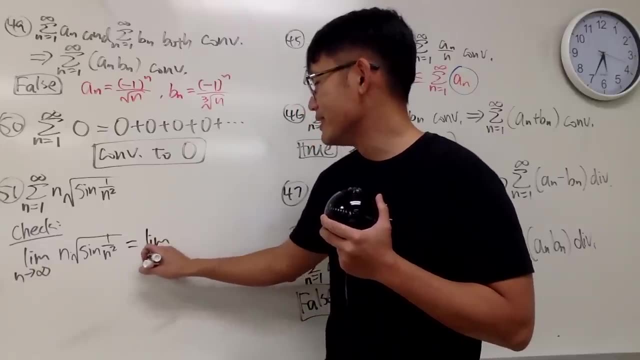 n times the square root of sine of 1 over n squared like this. Well, here's the deal. It's not so bad at all. This is n goes to infinity. Open the square root Because I can actually invite the n inside. 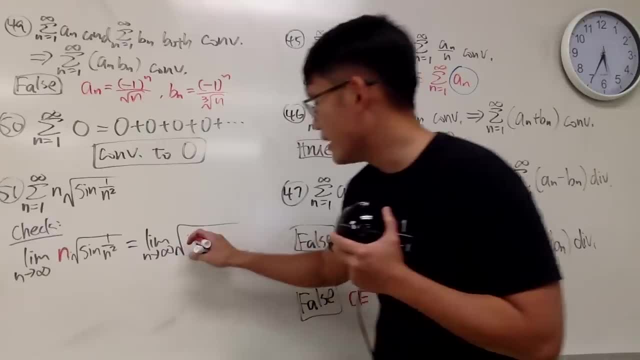 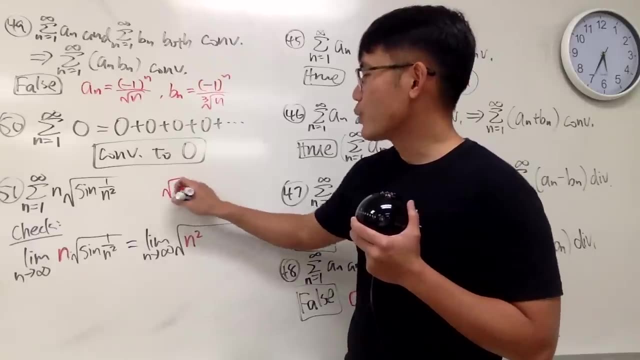 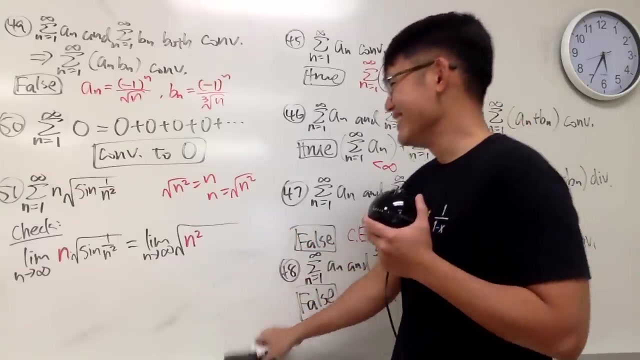 and it becomes. Let me just write this down, I will bring this n inside and it becomes n squared. All right, So you just kind of do the things backwards. Everybody knows square root of n squared is equal to n, But I know n is the same as square root of n squared. 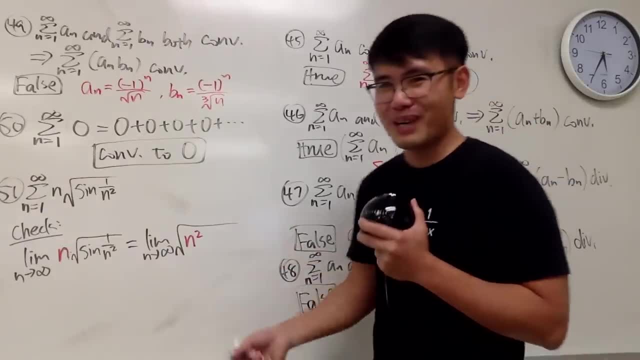 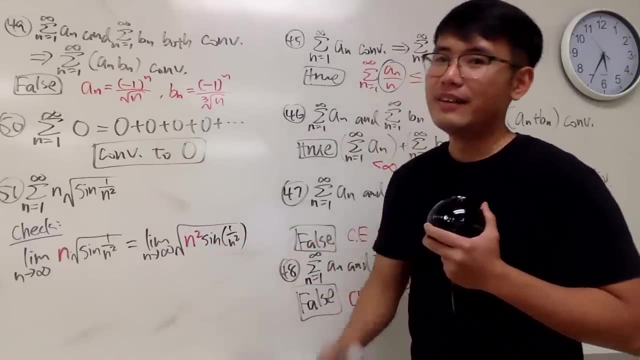 Don't you feel like a genius already when you do things like usual, things backwards, right, That's very nice, Okay. So here we have sine of 1 over n, squared like this. And now you know the deal: Bring this down down. 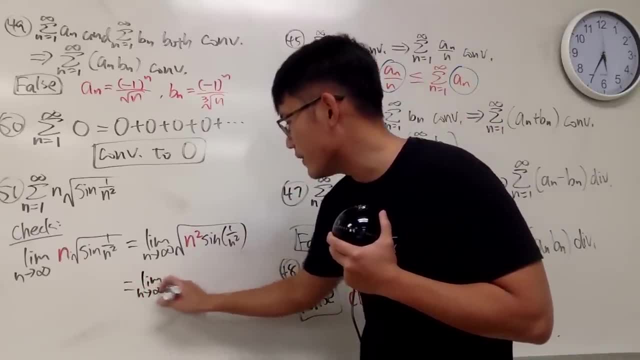 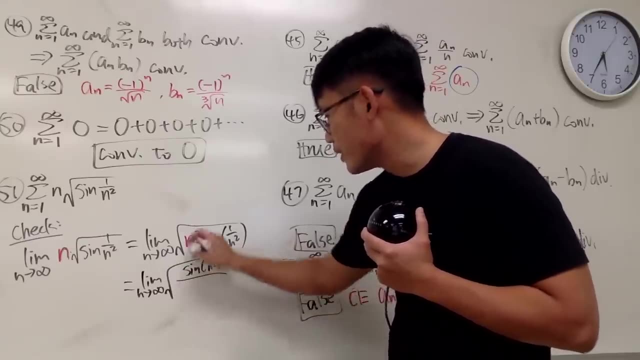 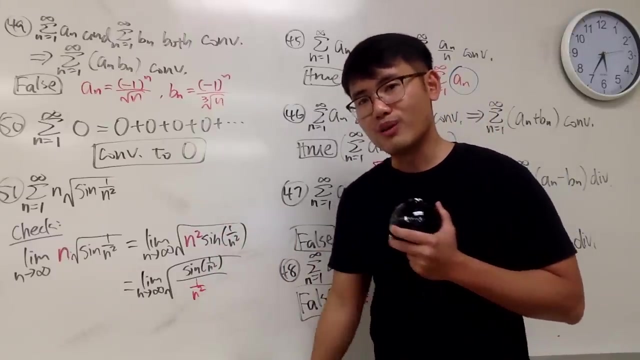 This right here is equal to the limit as n goes to infinity. Open the square root. This is sine of 1 over n squared, 1 over n squared over. Bring this down down. It becomes 1 over n squared, And the deal is that 1 over n squared does go to 0. 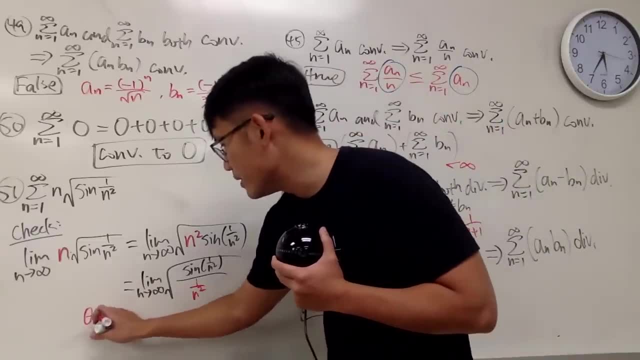 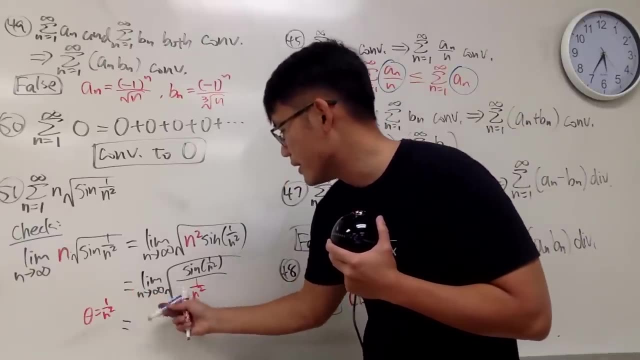 when n goes to infinity. So you can just take theta being 1 over n squared. So this right here is going to be the same as saying This is an h. This is the same as saying the limit as theta going to 0.. 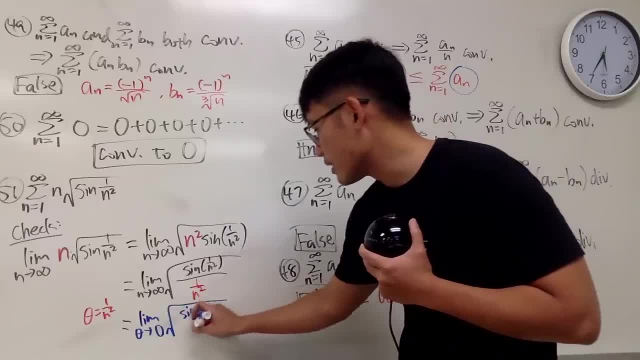 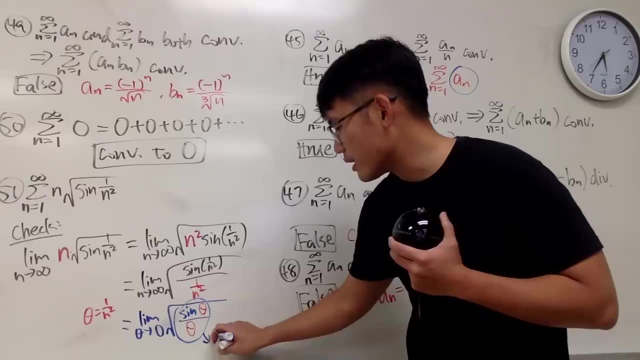 And we have the square root, And you have the sine of theta over theta, And the idea is that by the limit we know, this right here does go to 1. And we have the square root of 1.. So this all in all is just equal to 1.. 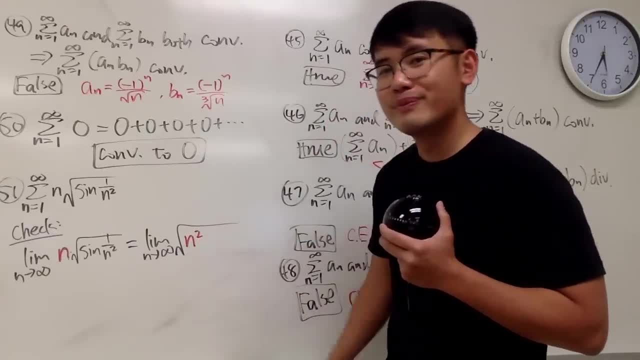 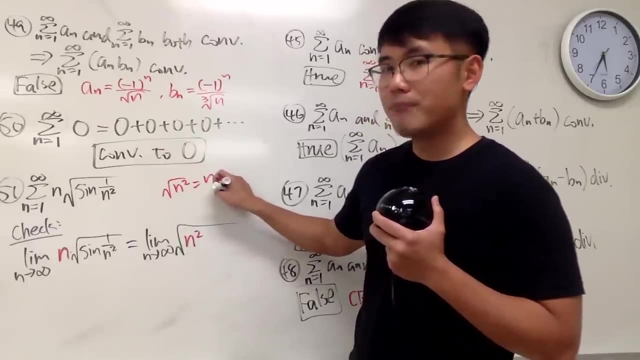 I'll bring this n inside and it becomes n squared. Alright, so you just kind of do the things backwards. Everybody knows square root of n? squared is equal to n, but I know n is the same as square root of n squared. 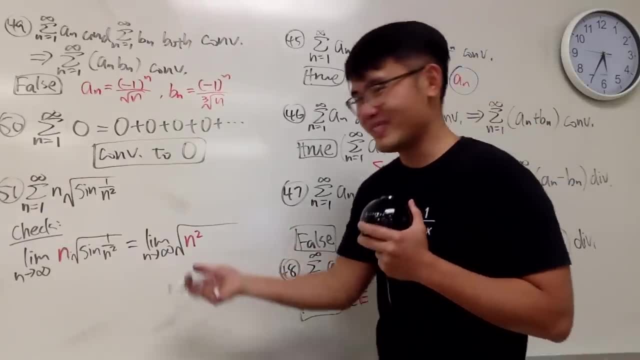 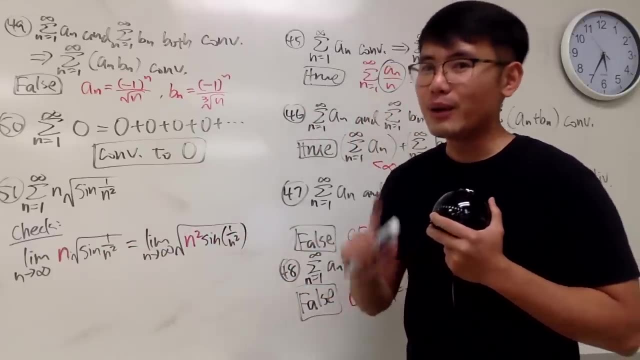 Don't you feel like a genius already doing things like usual, things backwards, right, That's very nice. Okay, so here we have sine of one over n squared like this. And now you know the deal: Bring this down down. 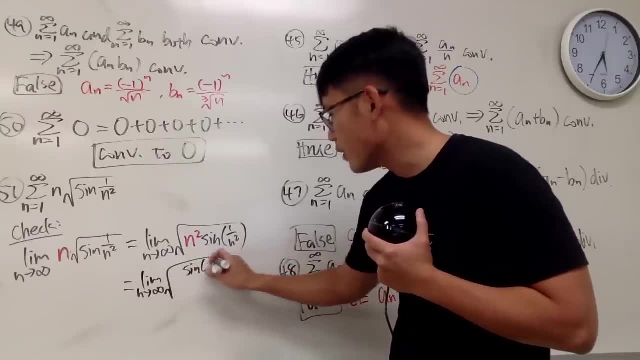 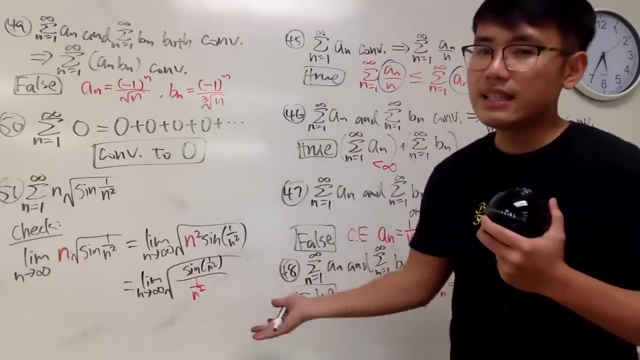 this right here is equal to the limit as n goes to infinity. open the square root. this is sine of one over n squared over. bring this down down, it becomes one over n squared and the deal is that n goes to infinity. 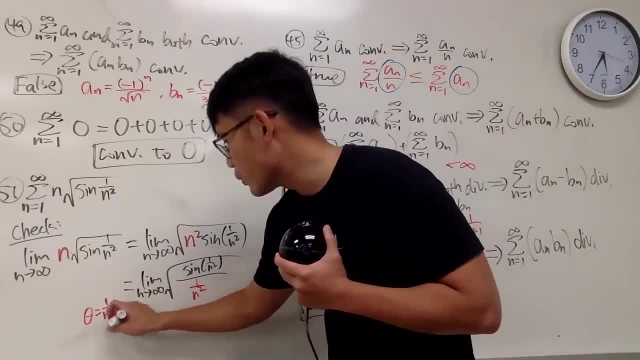 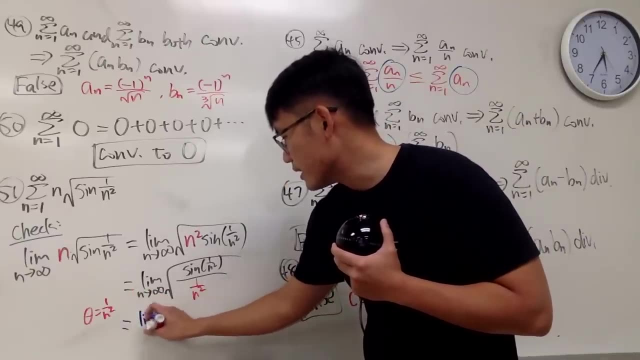 So you can just take theta being one over n squared. so this right here is going to be the same as saying this is an h, this is the same as saying the limit as theta going to zero and we have the square root. 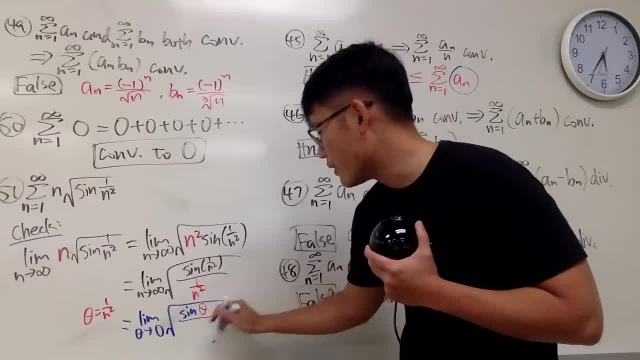 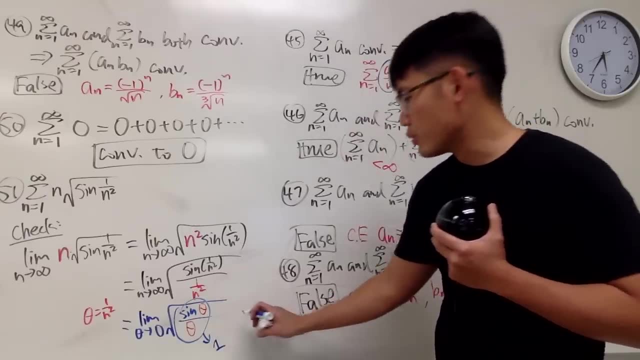 and you have the sine of theta over theta and the idea is that by the limit we know, this right here does go to one and we have the square root of one. it's just equal to one. One in test of divergence. 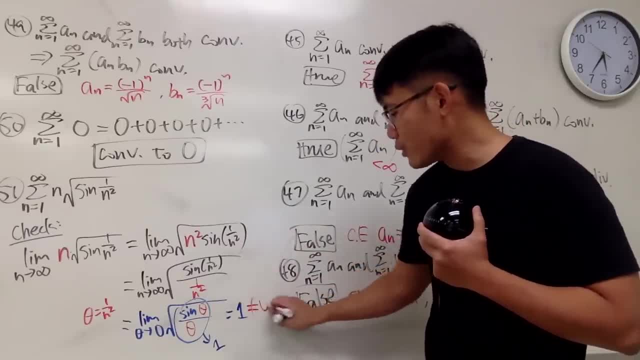 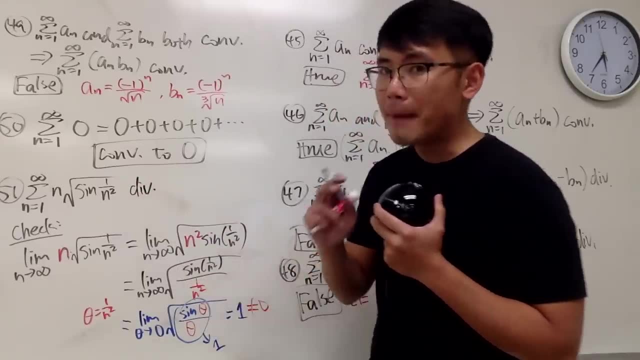 it's not good, Well, it's actually really good. this is not equal to zero. one is good, one is not equal to zero. so we can come back here and say this right here: divergence by the test for divergence: T, F, D. 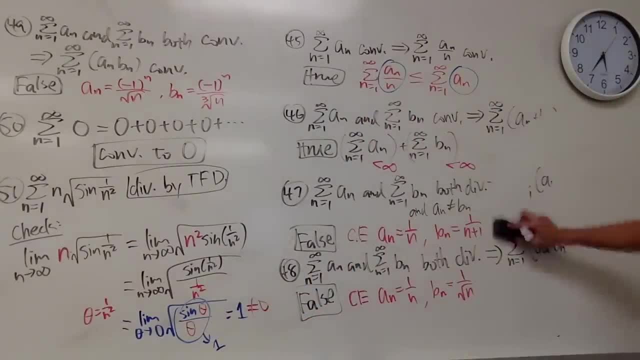 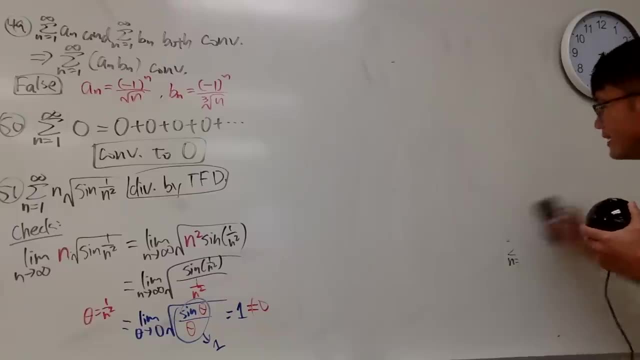 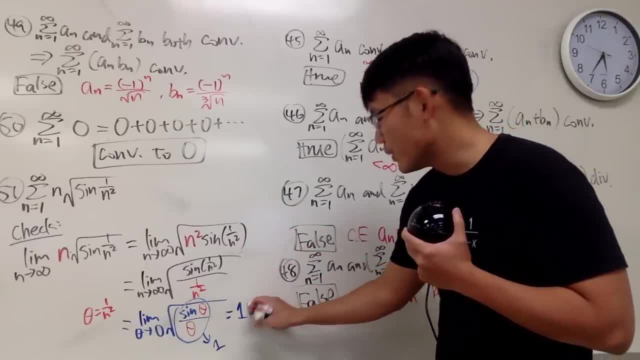 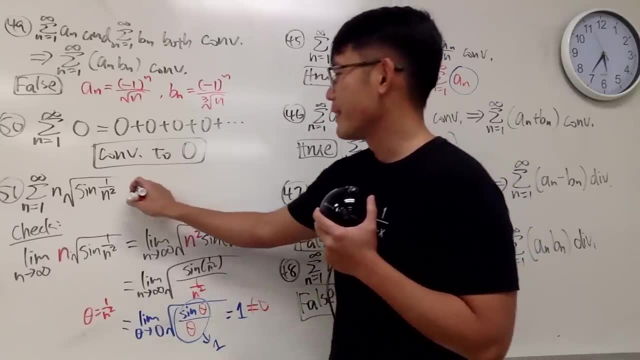 1 in test of divergence is not good. Well, it's actually really good. This is not equal to 0.. 1 is good. 1 is not equal to 0. So we can come back here and say this right here. 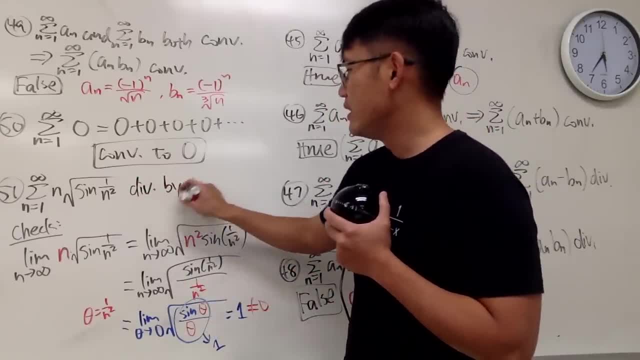 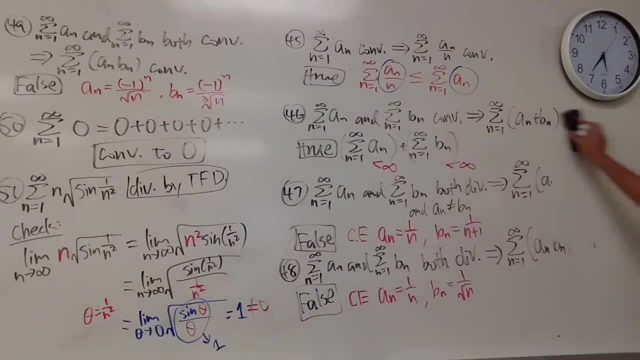 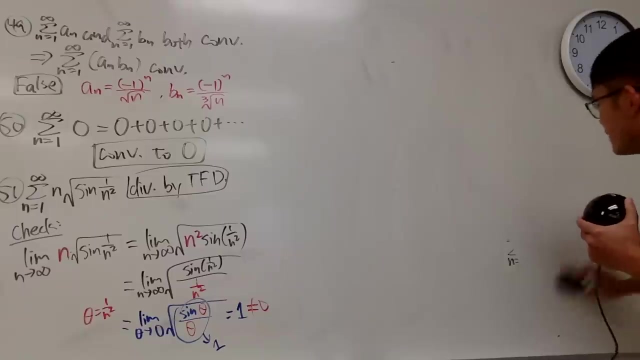 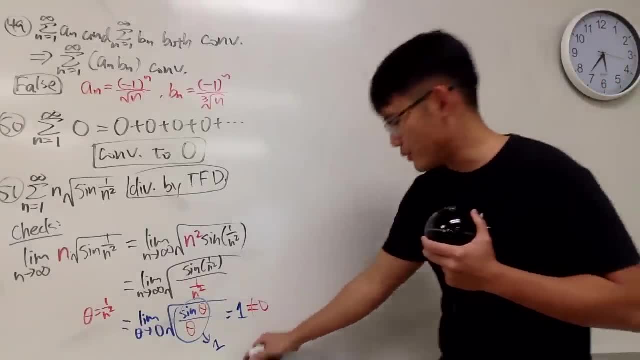 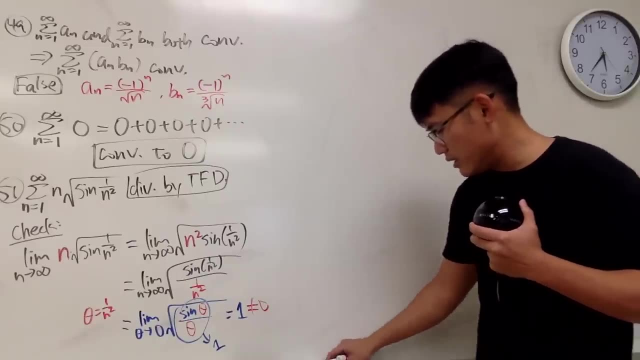 if you have to form some kind of a club or if you want to have to do some startup. if you don't have a name for it, just put T, F, D or L, C, T, L, C, T. 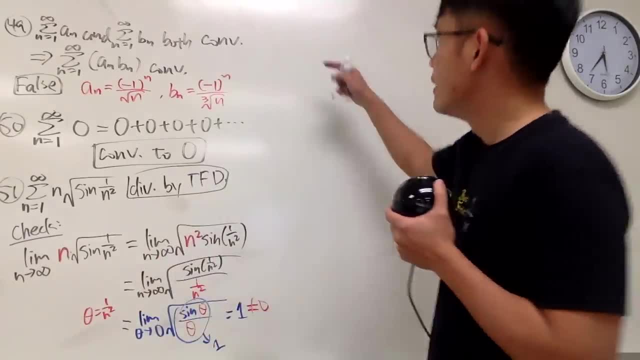 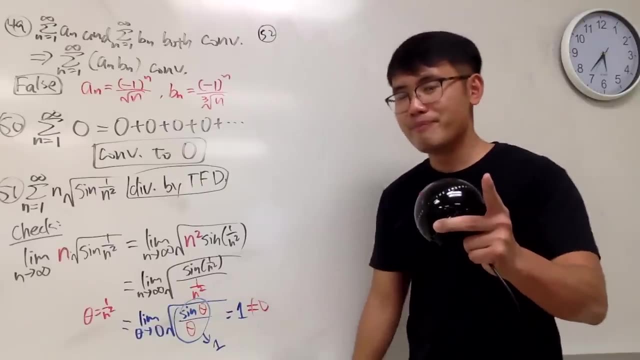 Okay, Number 52.. All right, So it's not a limit. I wish I'm taking a limit And yes, I will be doing 100 limit, but that may be in the summer, later on, later on, Okay. 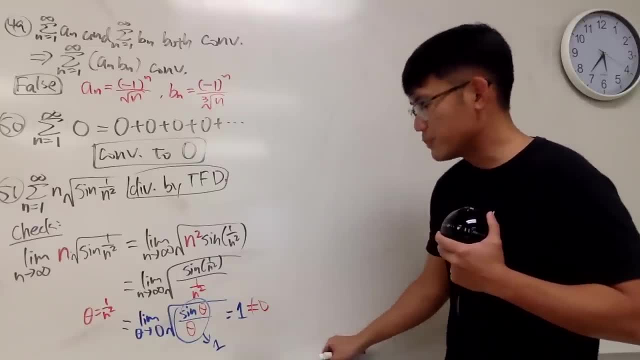 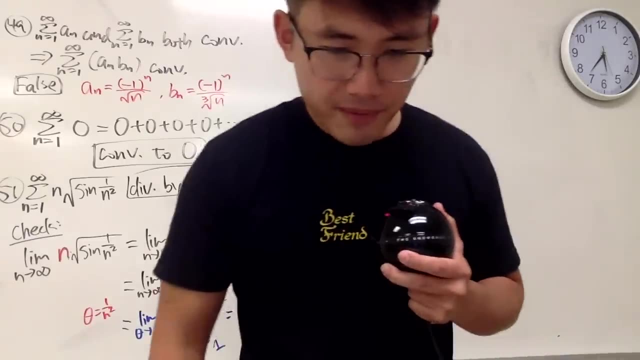 or if you want to have to do some startup, if you don't have a name for it, just put T, F, D or L, C, T, L, C, T. Okay, number 52. So it's not a limit. 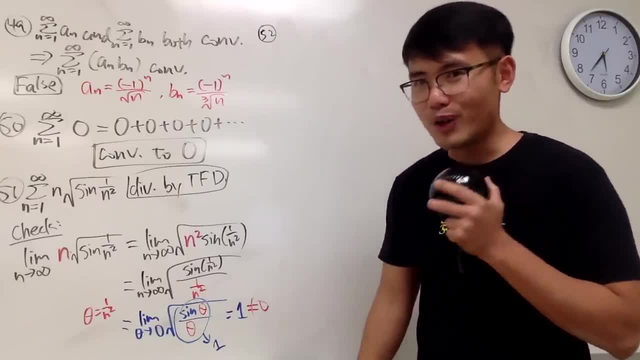 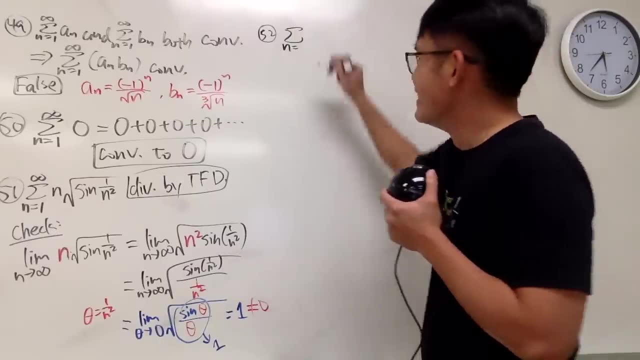 I wish I'm taking a limit and, yes, I will be doing 100 limit, but that may be later on, later on, later on. okay, Don't, don't, don't, John, later on, later on. 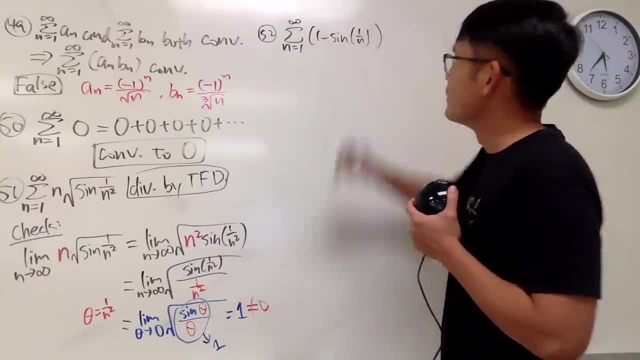 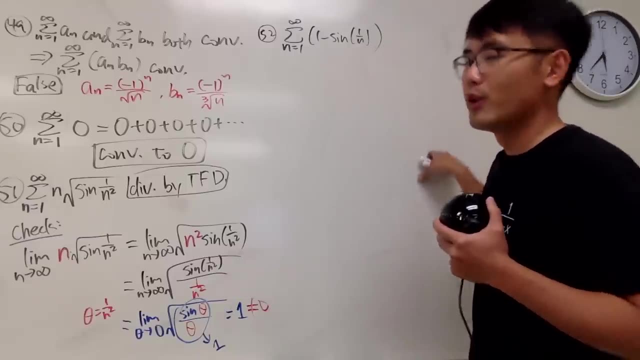 I'm sorry that I'm not. I don't have the time to do that this semester, but next semester, hopefully, Let's see what happens. 1 minus sine of 1 over N, This right here, very nice, It's just divergence. 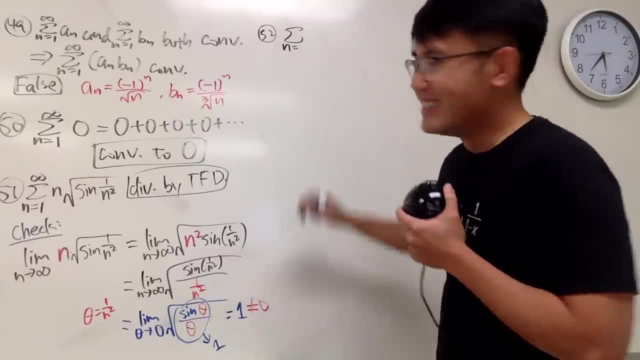 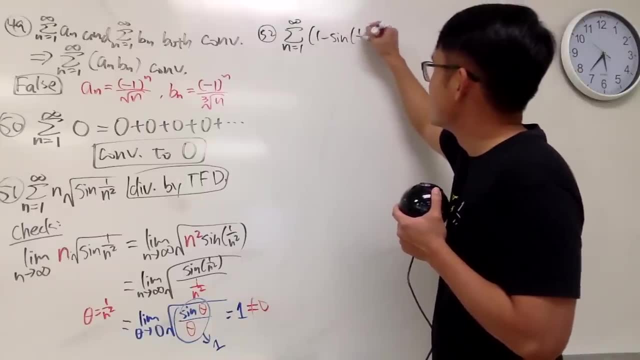 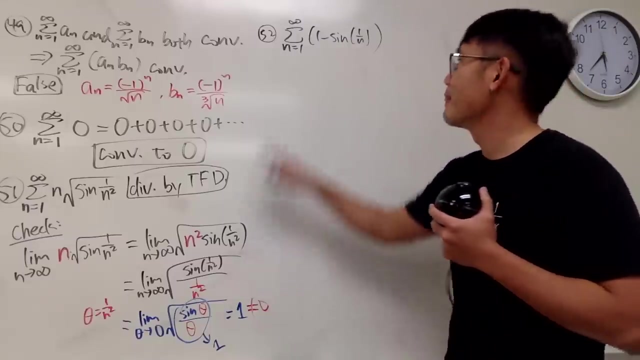 Don't, don't, don't Later on. I'm sorry that I'm not. I don't have the time to do that this semester, but next semester, hopefully, Let's see what happens. 1 minus sine of 1 over N. 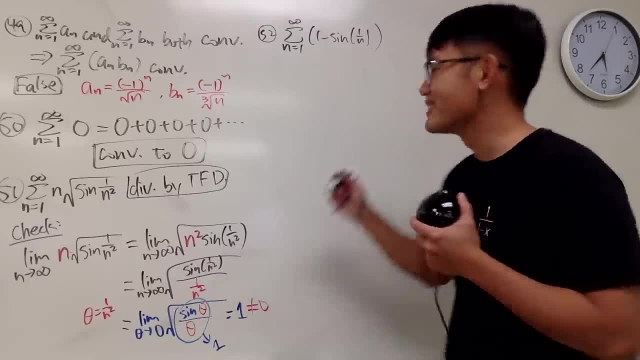 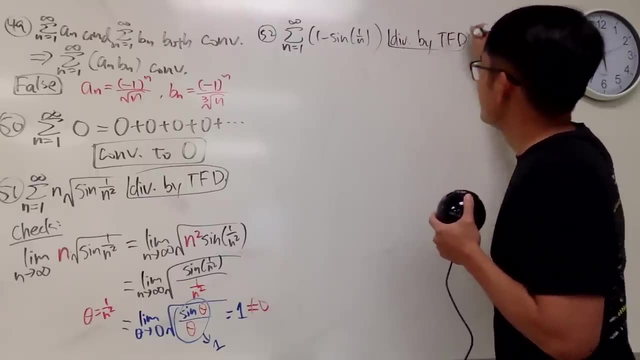 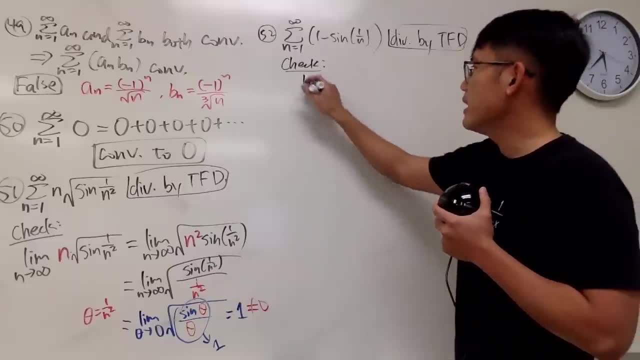 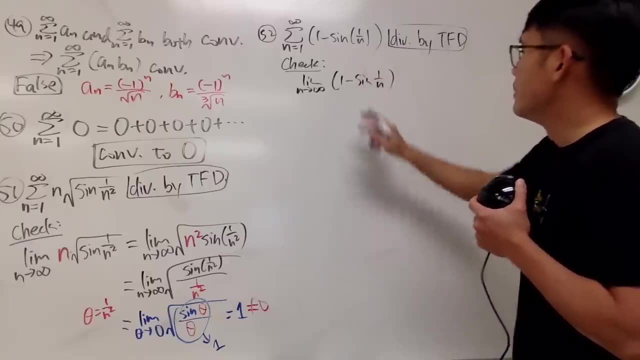 It's pretty much just that. Now let's go ahead and check. If we take the limit as N goes to infinity, this is just going to be 1 minus sine of 1 over N. Put the infinity in here, so we get 1 minus sine of 1 over infinity. 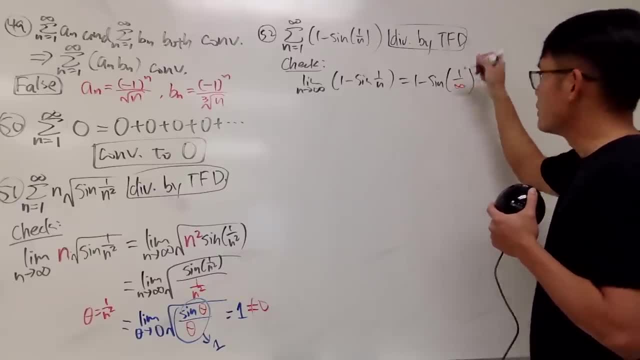 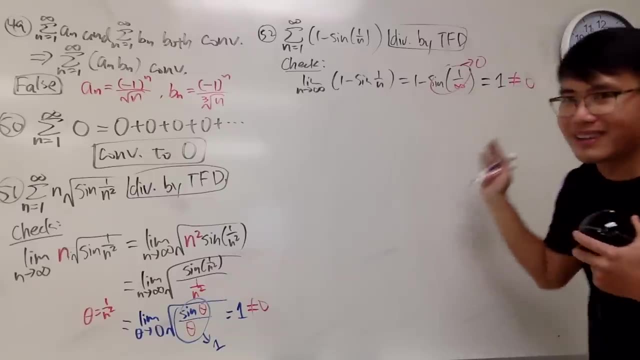 Which this guy is 0. The whole thing sine of 0 is 0. So this right here does give us 0. All in all we get 1.. But 1 is not the same as 0. So we are done. 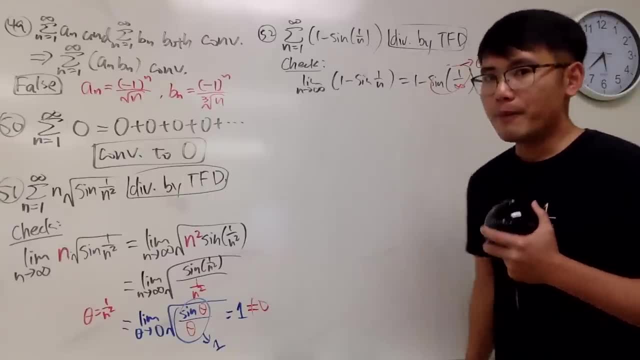 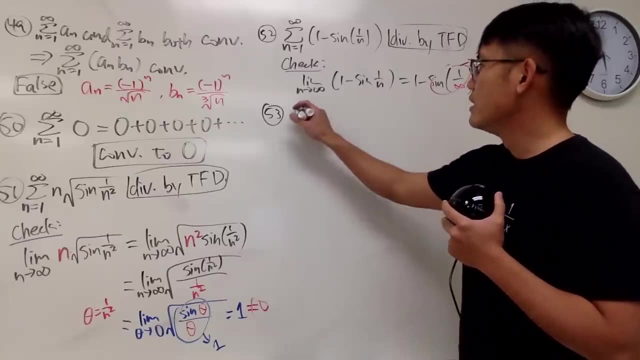 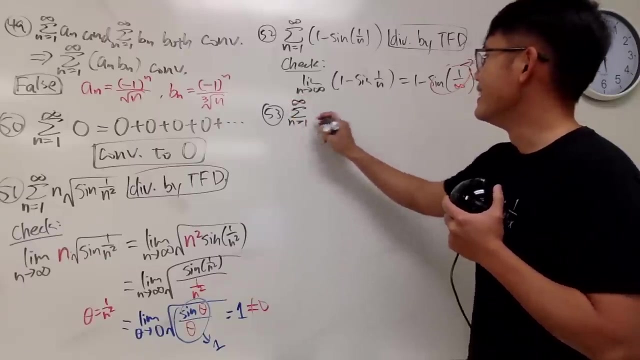 T F D for the win. Seriously, Now to make things more serious: T F D is 3.. What if we have cosine instead? The sum as N goes from 1 to infinity and then 1 minus. 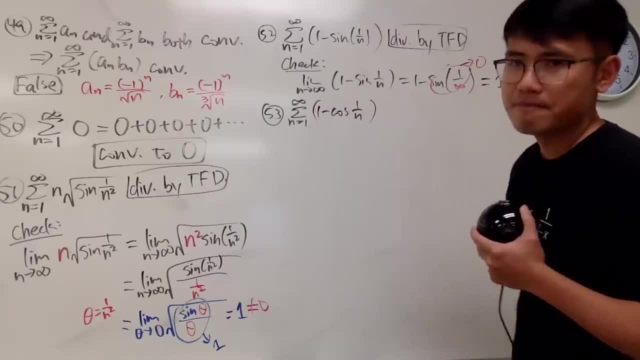 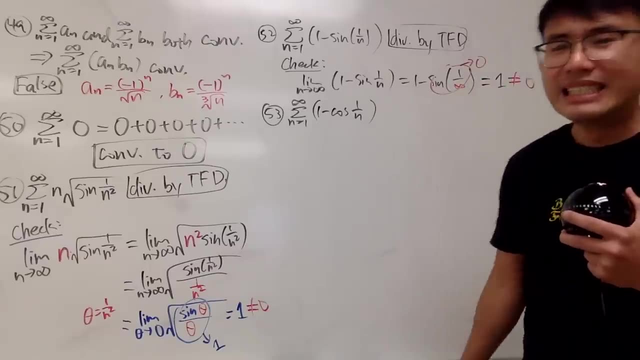 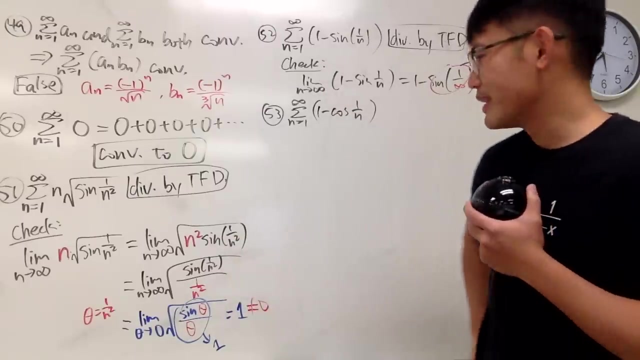 cosine of 1 over N like that. Unfortunately, if you have cosine, the cosine of 0 is 1.. 1 minus 1 is 0.. T F D doesn't work in this case. I know I feel sad too. 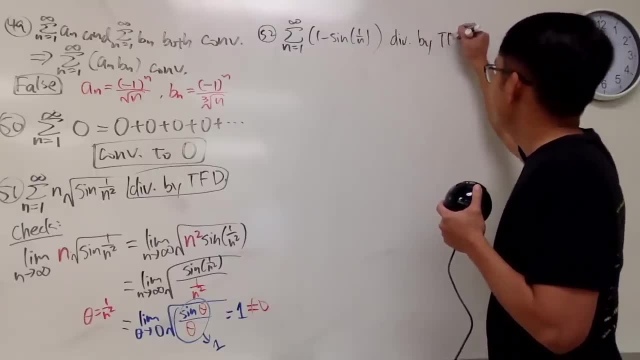 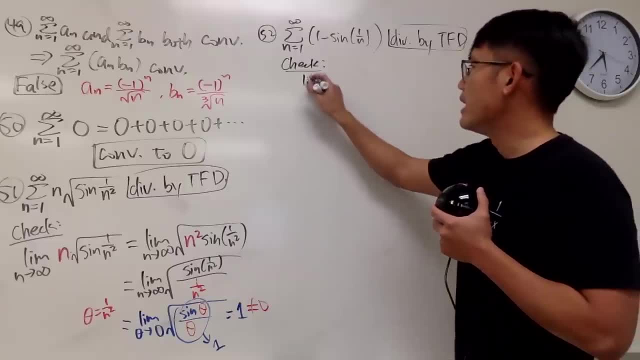 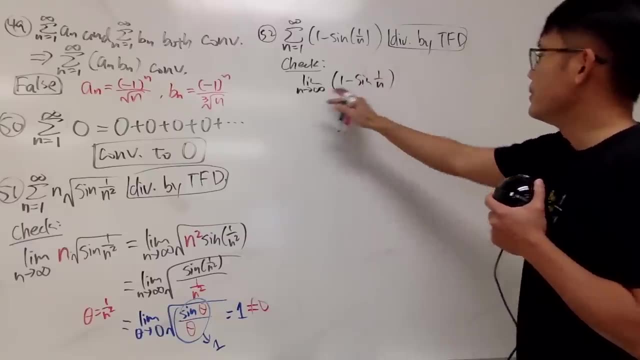 Now let's go ahead and check. If we take the limit as N goes to infinity, this is just going to be 1 minus sine of 1 over N. Put the infinity in here, so we get 1 minus sine of 1 over. 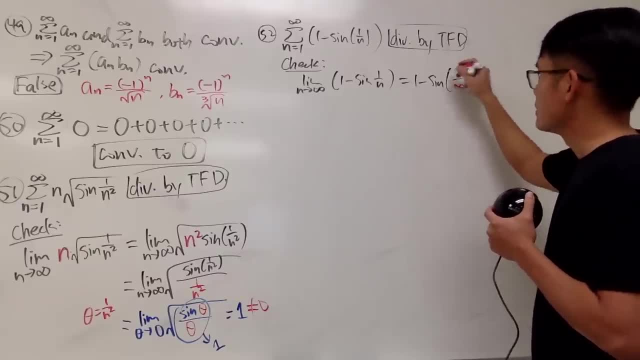 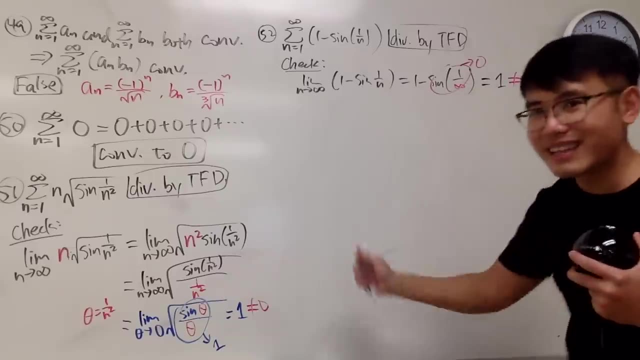 infinity, which this guy is 0. The whole thing sine of 0 is 0, so this right here does give us 0. We get 1, but 1 is not the same as 0, so we are done. 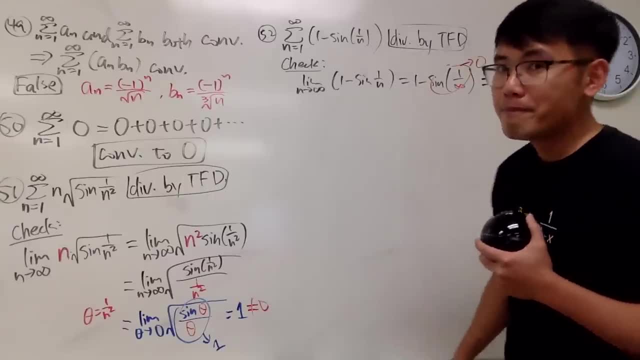 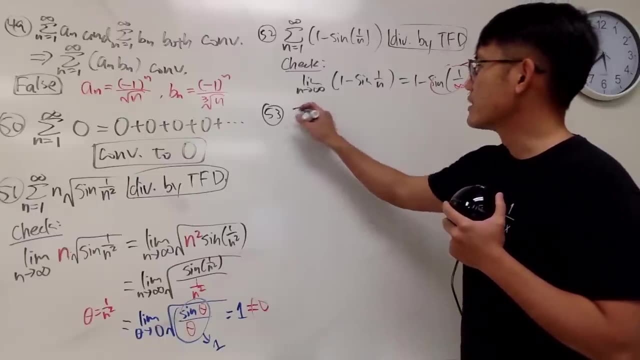 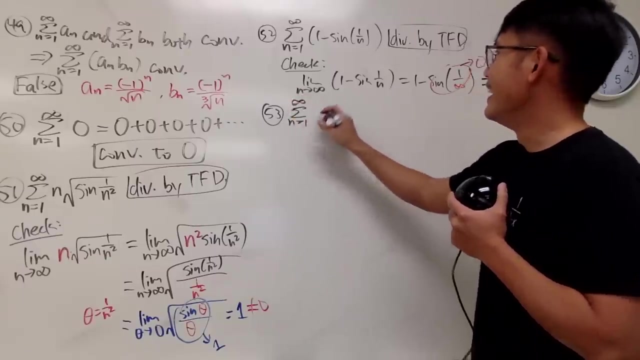 T F D for the win. seriously, Now to make things more serious: T F D is 3.. What if we have cosine instead? The sum as N goes from 1 to infinity and then 1 minus. 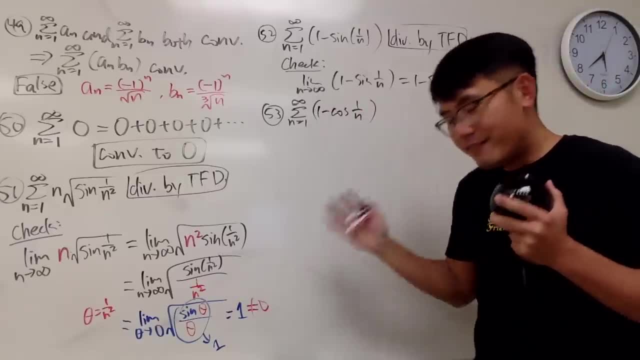 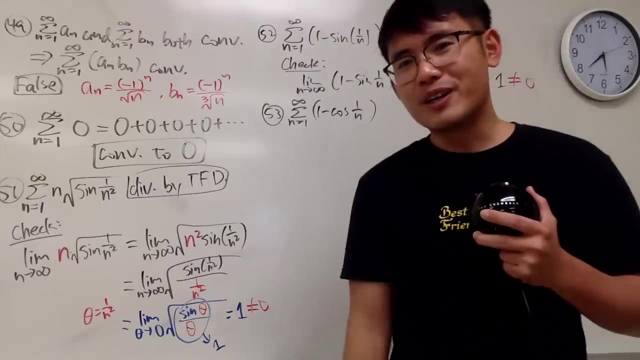 cosine of 1 over N, like that. Unfortunately, if you have cosine, cosine of 0 is 1, 1 minus 1 is 0.. T F, D doesn't work in this case. I know I feel sad too. 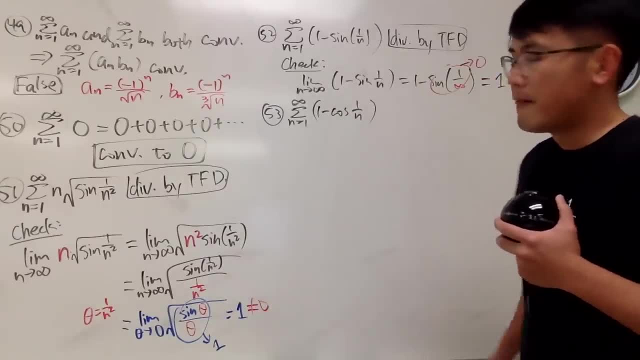 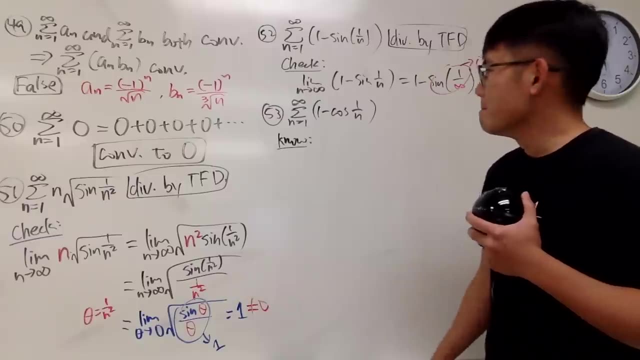 But it's okay, We can handle this, No big deal. First let me just show you guys what we can do right here. Let's put down what we know, Okay? So if you put down the sum as N goes from 1 to infinity, 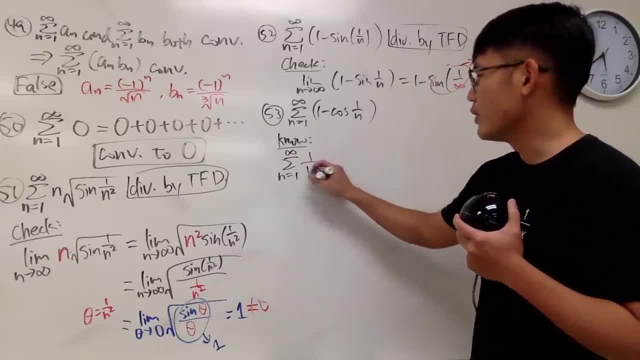 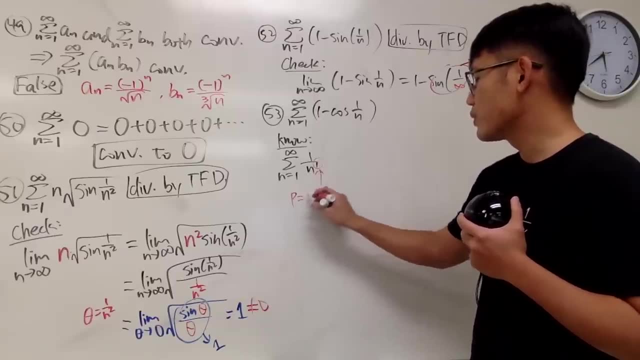 you see 1 over N. Maybe you want to use the limit comparison test with 1 over N, right here, right, So okay, sure, This right here is 1 over N, which is P is equal to 1,, which is less than or equal to 1.. 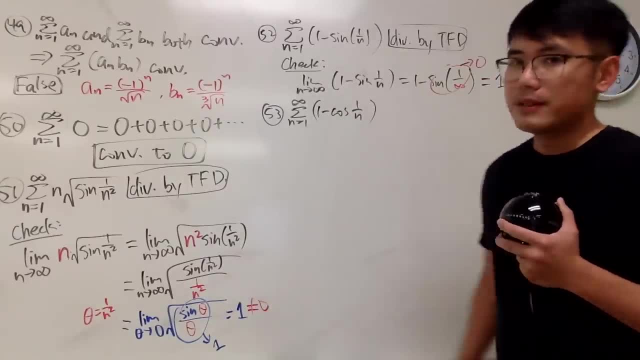 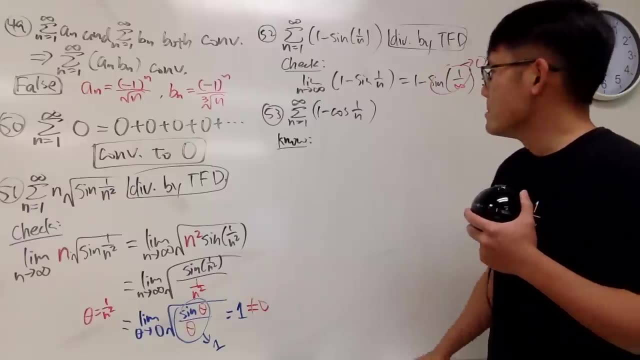 But it's okay, we can handle this, no big deal. First let me just show you guys what we can do right here. Let's put down what we know. Okay, so if you put down the sum as N goes from 1 to infinity, 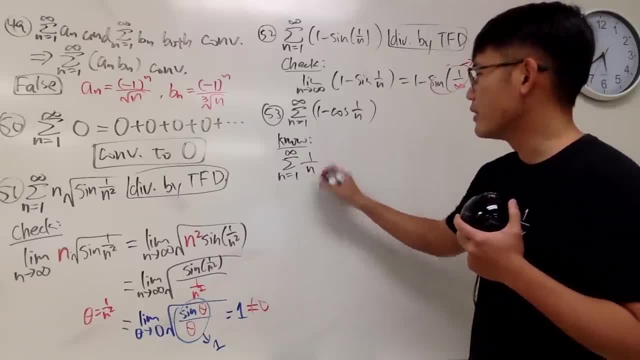 you see 1 over N. maybe you want to use the limit comparison test, which is 1 over N, right here, right? So okay, sure, this right here is 1 over N, which is P is equal to 1,. 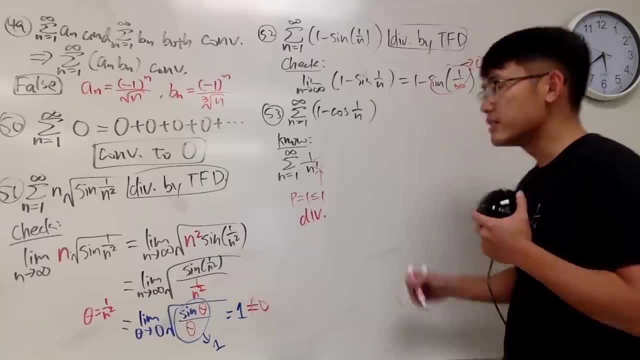 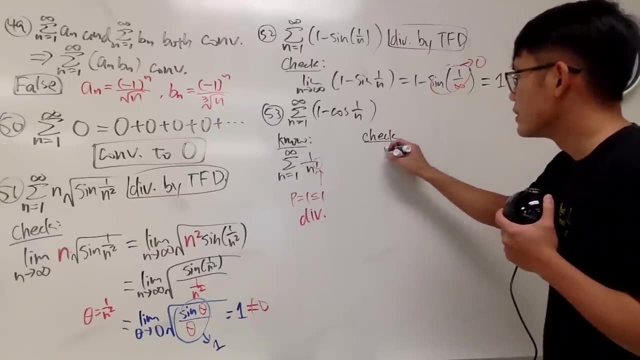 which is less than or equal to 1.. Okay, okay, okay, So it diverges. Okay, okay, But let's take this right here. Let's go ahead and check the limit. Put the one that you're doing on the top. 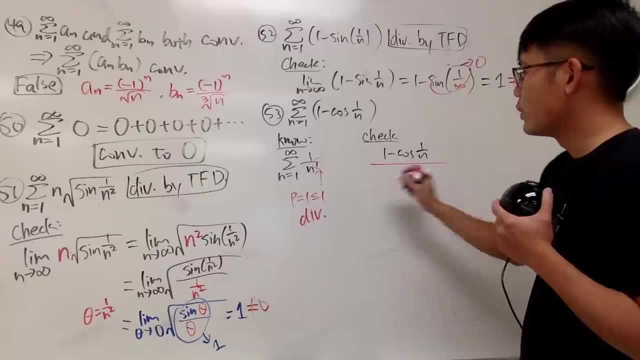 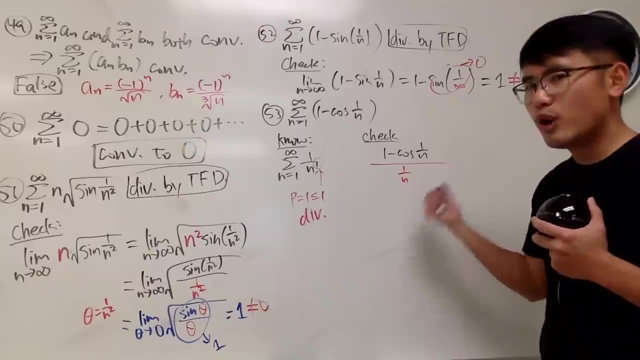 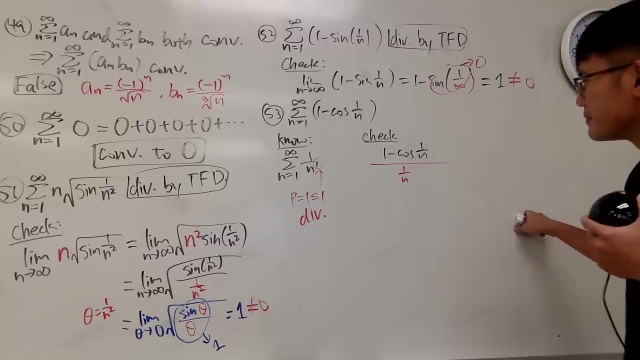 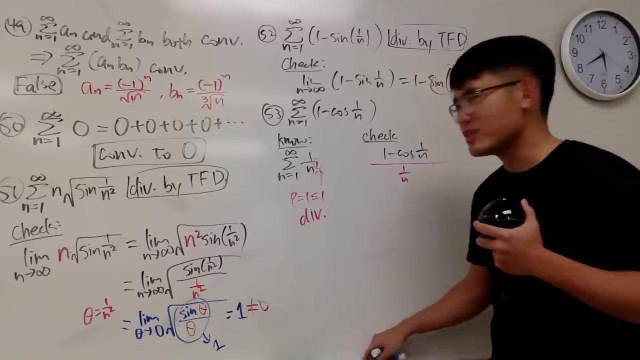 which is 1 minus cosine of 1 over N over the one that we have to do on the bottom, which is 2 minus cosine of 2 over N over N, over R times plus 2� times 0. Yes, So it's. 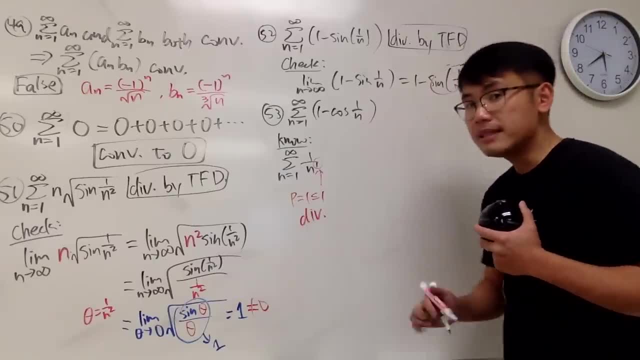 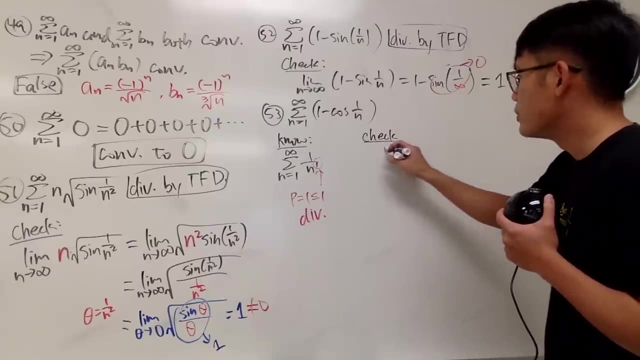 Okay, okay, okay, So it diverges. Okay, okay, But let's take this right here. Let's go ahead and check the limit. Put the 1 that you're doing on the top, which is 1 minus cosine of 1 over N. 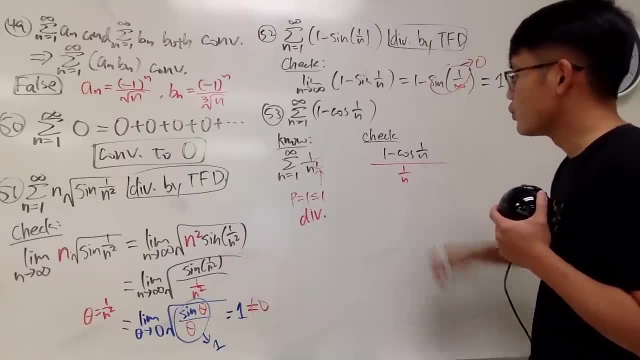 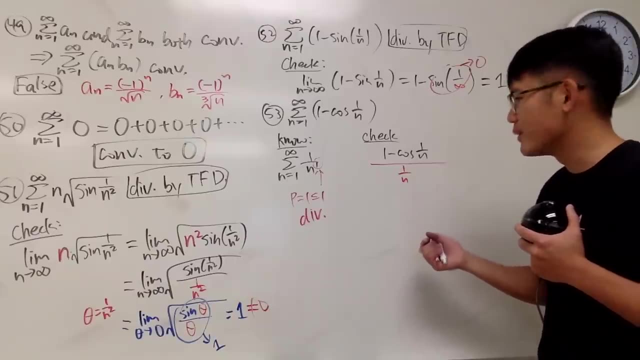 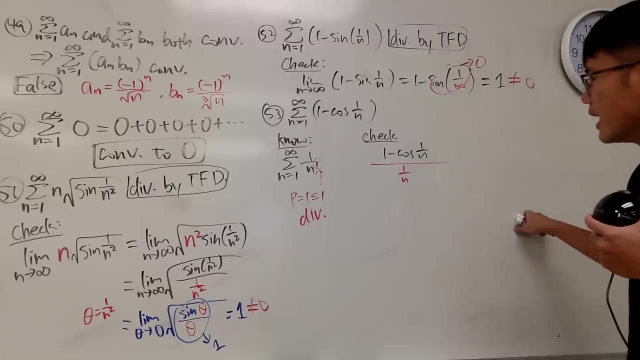 over the 1 that we have to do on the bottom, which is 1 over N, like this: Hmm, This is a 0 over 0 situation. huh, Right, So huh, and then it's not really anything that we know, huh. 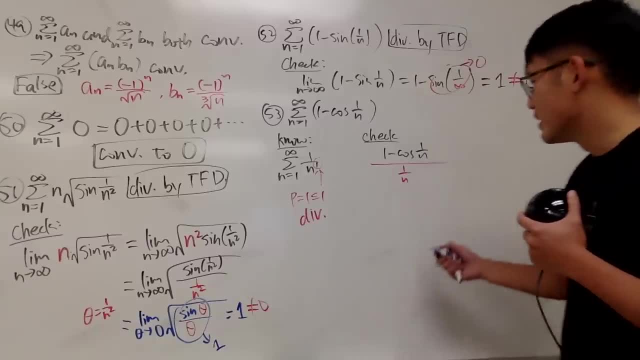 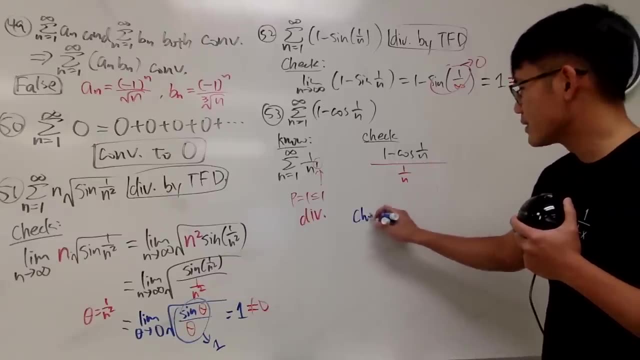 And it's like we have to do the Lapithos rule. So I will actually do this. We actually have to change this to x so that we can take the derivative model. So I will just check. So this right here is just my check in blue. 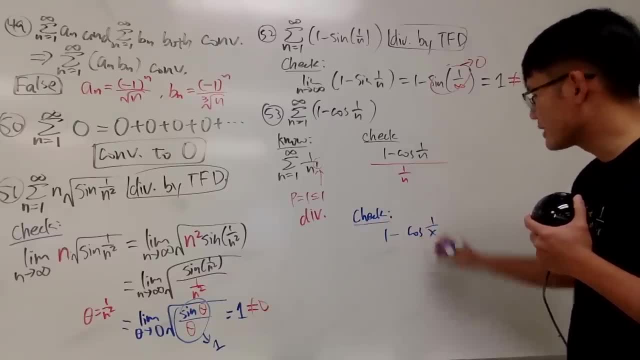 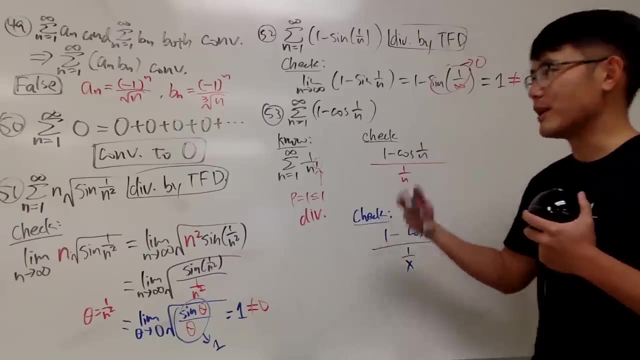 1 minus cosine of 1 over x. And the reason I changed it to x is because ddN technically doesn't make sense, okay, And it's supposed to just be a whole number. so yeah, Anyway, Lapithos rule in action. 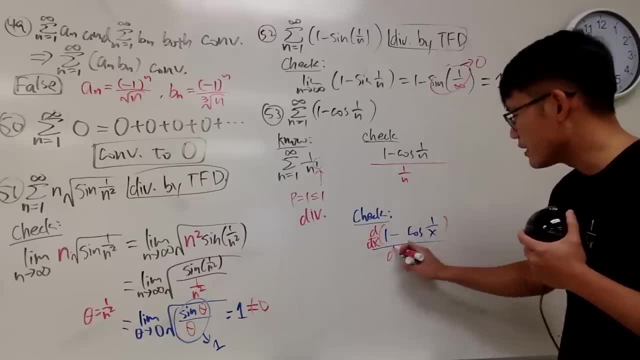 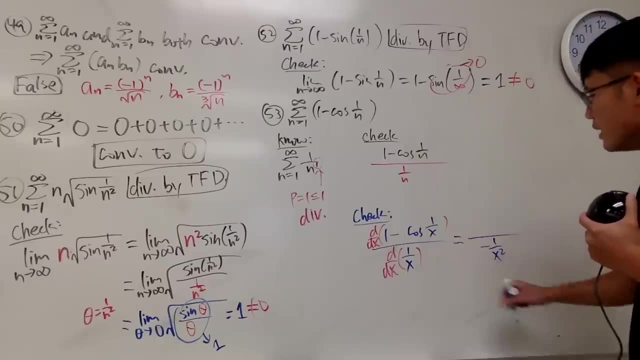 because this is a 0 over 0 situation. So I'm going to differentiate the top and also differentiate the bottom. Let's see if this works or not. Differentiate the bottom: we get negative 1 over x squared. Differentiate the top: 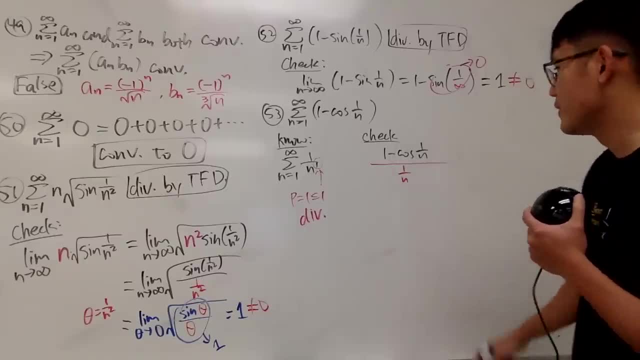 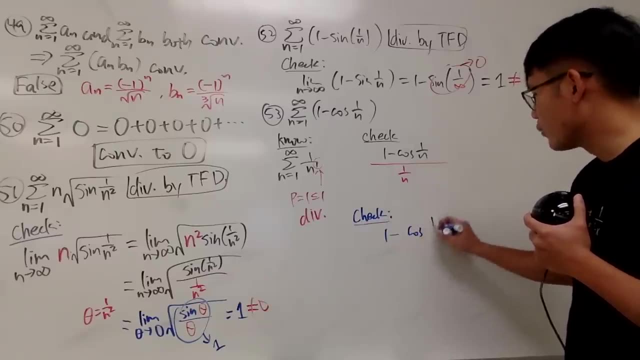 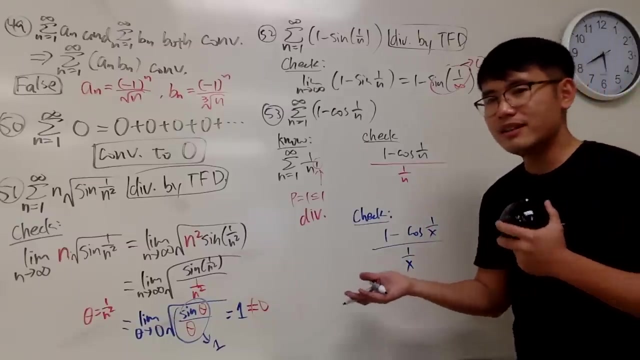 1 over N over 1 over 2 times 6 plus 4 times x, and the reason I changed it to x is because ddn technically doesn't make sense, okay, and it's supposed to just be a whole number, so yeah, 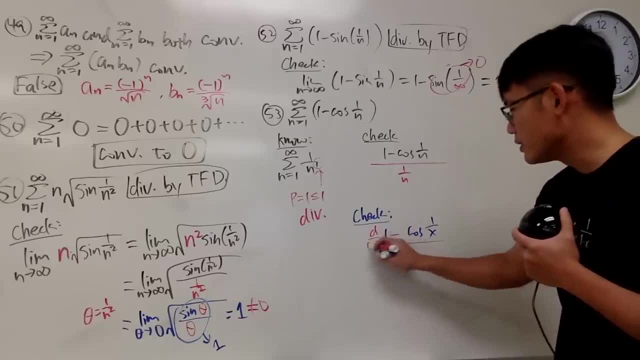 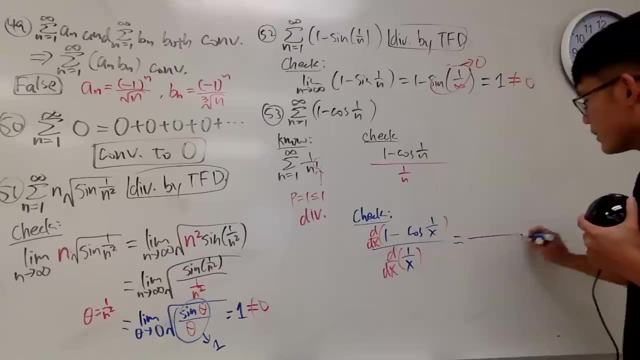 Anyway L'Hopital's rule in action, because this is a 0 over 0 situation. so I'm going to differentiate the top and also differentiate the bottom. let's see if this works or not. Differentiate the bottom: we get negative 1 over x squared. differentiate the top: the. 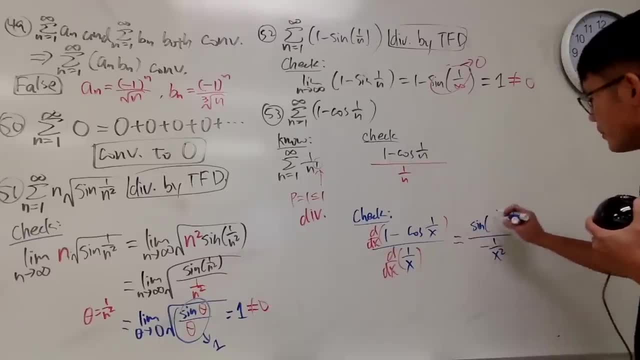 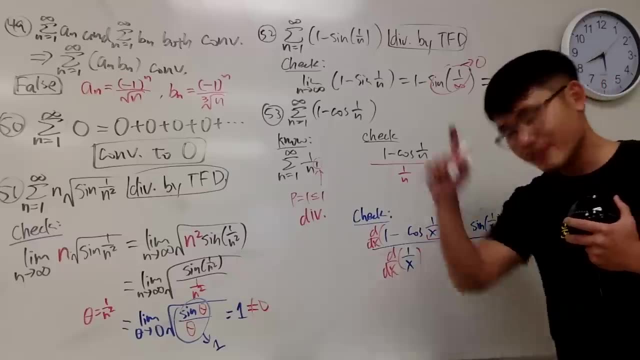 derivative of negative cosine is positive sine. so that's good. and then we have the input is 1 over x times. okay, the derivative of the inside. because of the Chengdu- oh my god, first time saying Chengdu today, that's so cool. here we get negative 1 over x squared. 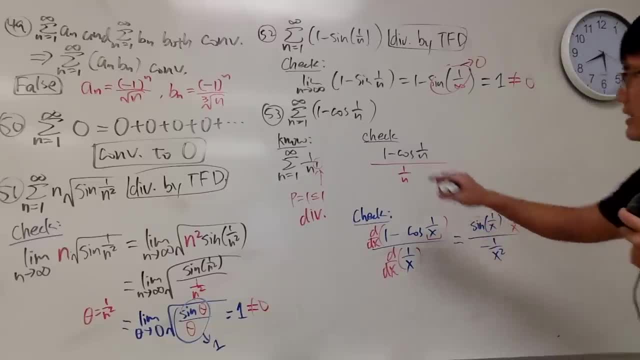 Here's the problem: cancel, cancel as x right. this right here is technically as x goes to infinity. this right here actually go to 0, cancel cancel sine of 0 is 0.. Let me tell you this is upsetting. for the first time, this right here does not work. 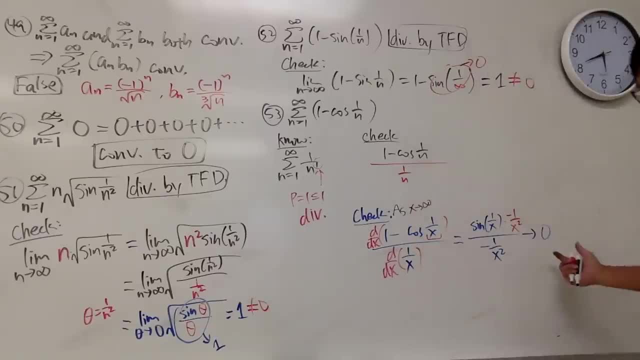 The idea is that when we are doing the limit comparison test, 0 is actually a sad face, 0 is actually a sad face for limit comparison test. so unfortunately this right here does not help and I know how you guys feel, but we really have to just kind of cross this. 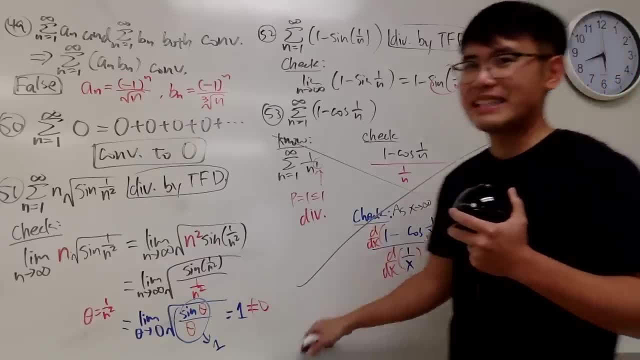 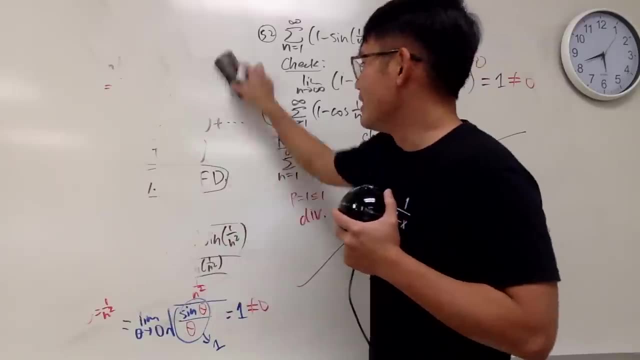 out. but it doesn't mean that you cross this out on the exam and expect you can get full credit. It's just that we have to come back to like another part of your paper and do more work to figure that out. 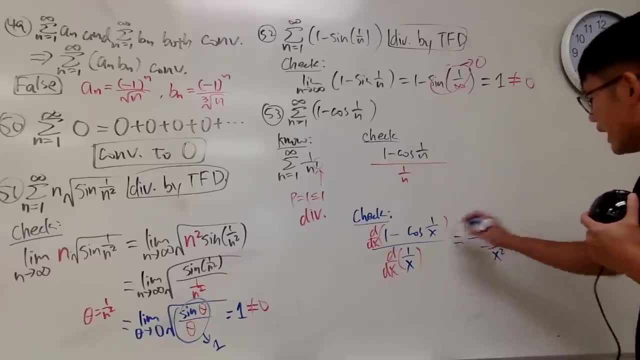 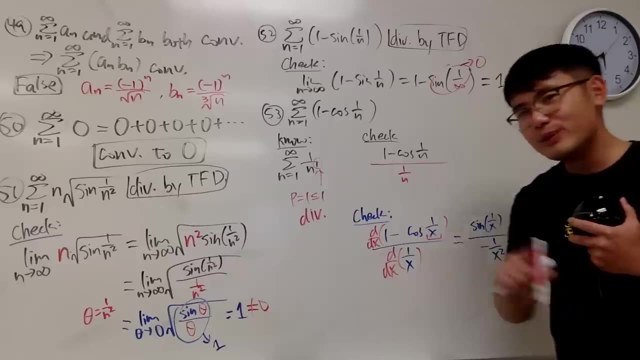 the derivative of negative cosine is positive sign, so that's good. And then we have: the input is 1 over x times, okay. the derivative inside because of the Chengdu. Oh my god, first time saying Chengdu today. That's so cool. 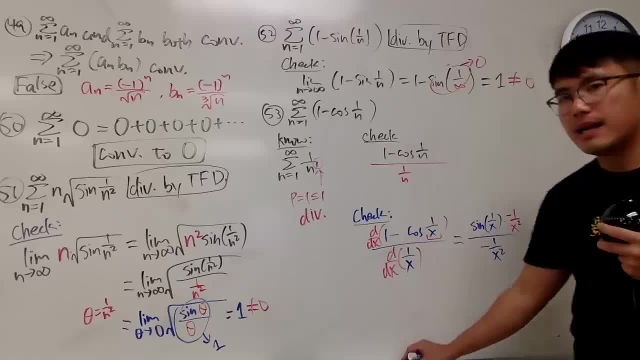 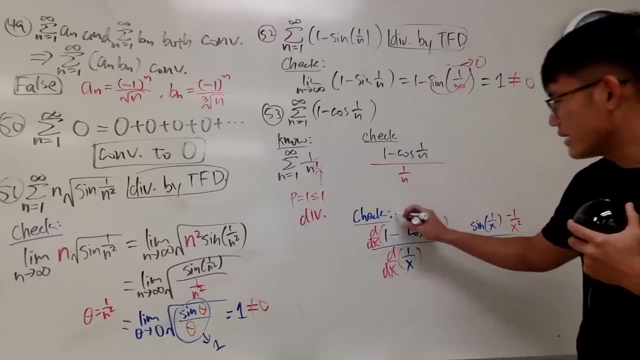 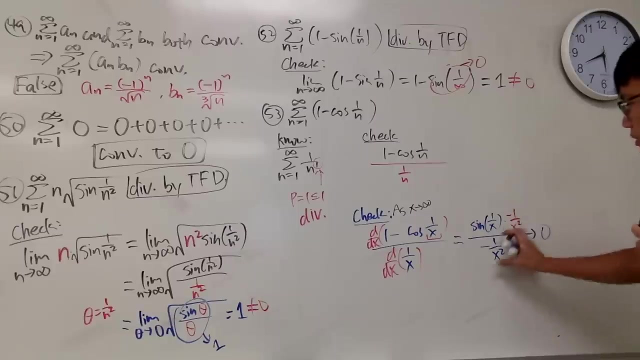 Here we get negative 1 over x squared. Here's the problem. Cancel, cancel as x right. This right here is technically as x goes to infinity, This right here actually goes to 0.. Cancel, cancel. sine of 0 is 0.. 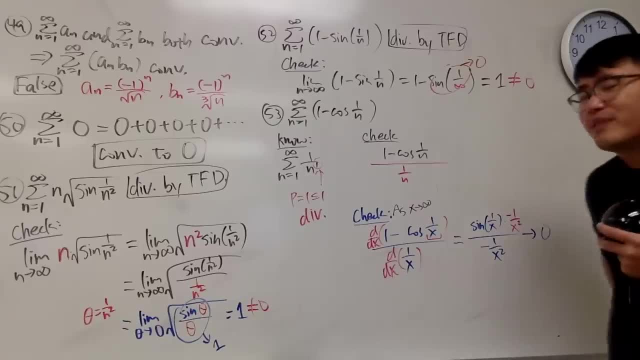 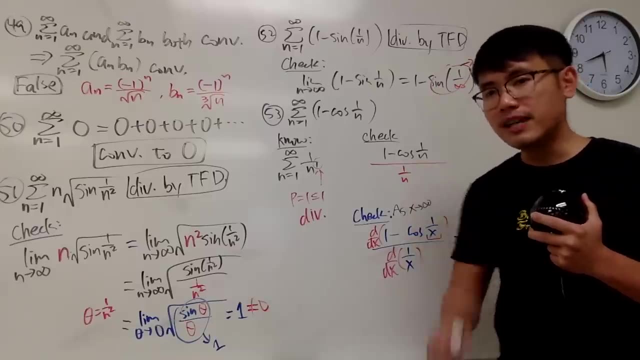 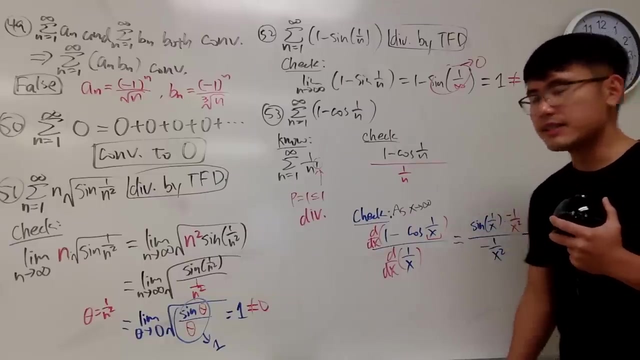 Let me tell you this is upsetting for the first time. This right here does not work. The idea is that when we are doing the limit comparison test, 0 is actually a sad face, 0 is actually a sad face for limit comparison test. 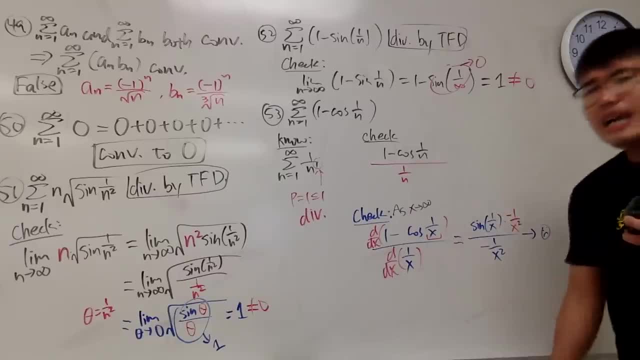 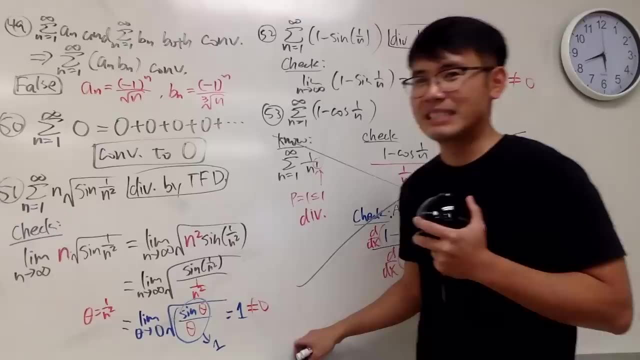 So unfortunately this right here does not help And I know how you guys feel, but we really have to just kind of cross this out. But it doesn't mean that you cross this out on the exam and expect you can get full credit. 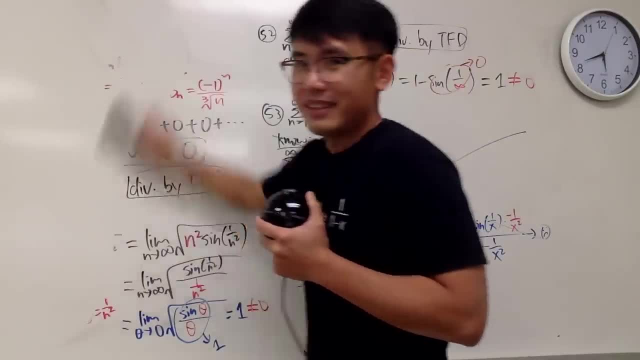 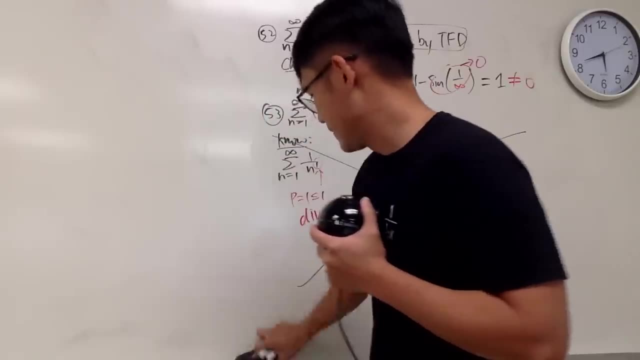 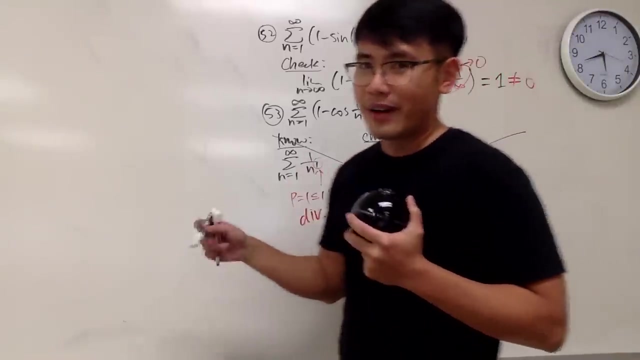 It's just that we have to come back to like another part of your paper and do more work to figure that out. Okay, so this right here didn't work and we just have to do it again Like 53.. Just don't give up. 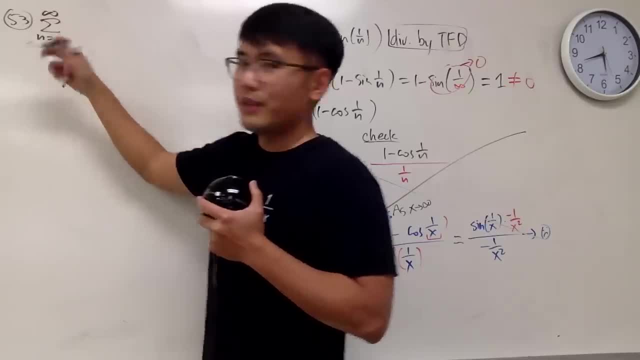 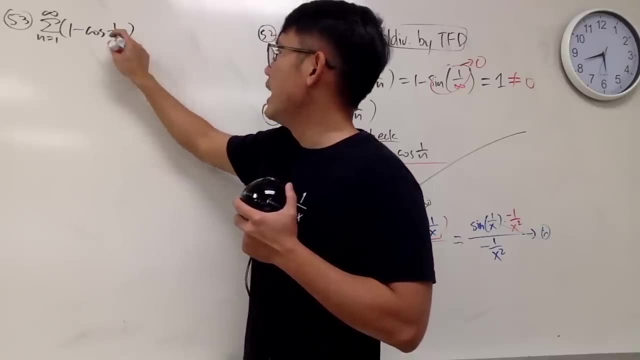 And my questions on the exams will be fair enough. so if you just really think about it, if you're really prepared, you should be able to handle this kind of things. Oops, not x, it's n right here. Okay, here we go. 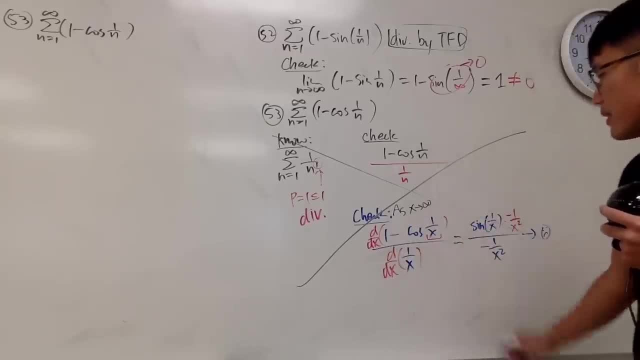 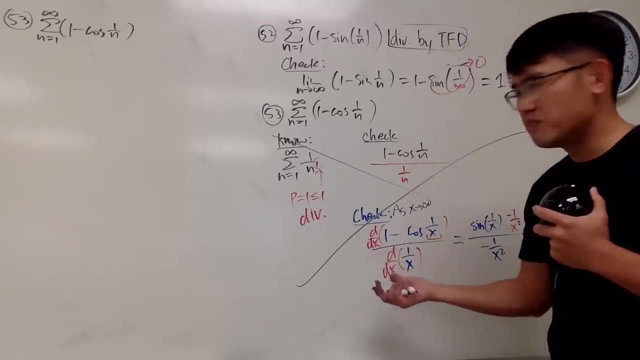 Seriously, you guys will see why this doesn't imply anything. okay, Because this right here diverges. If this is 0, imagine 0 divided by infinity. You can have infinity over infinity still 0, or finite over infinity to be 0,. 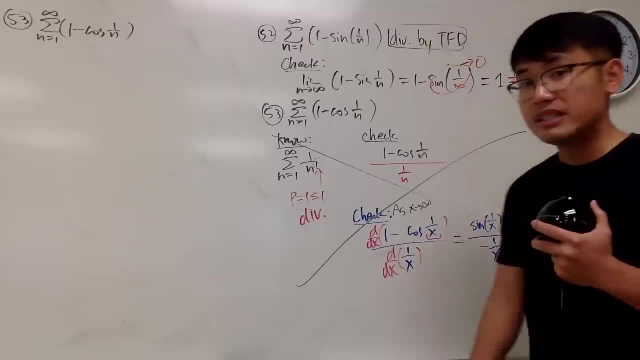 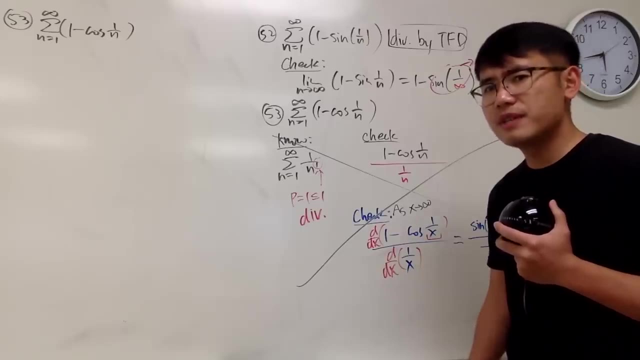 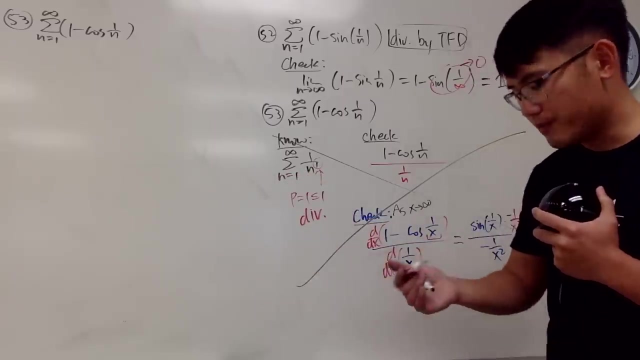 so you cannot really draw a conclusion. That's why 0 is not helping us at all in this case. Maybe it converges, because again, if you do this, divided by that, that was a divergent. So let me try the other one. 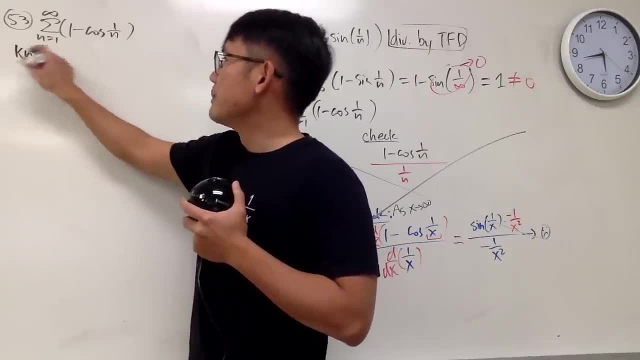 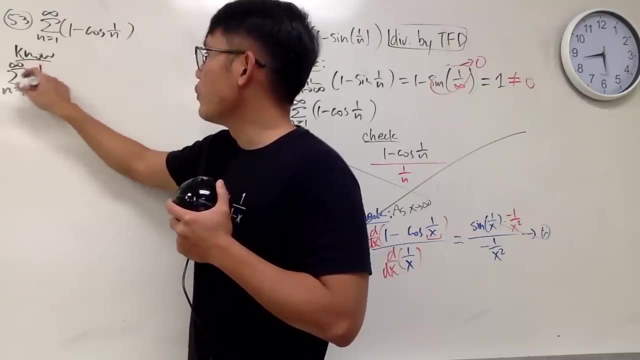 Let me try the other one. So suppose we do the following. Suppose I want to use the sum, as n goes from 1 to infinity, of 1 over n squared. Let me try the convergent version, which is: p is 2,. 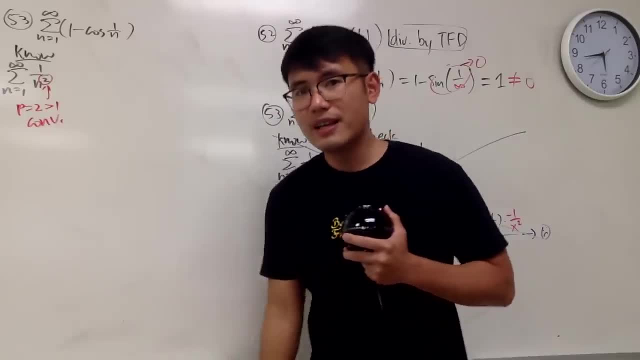 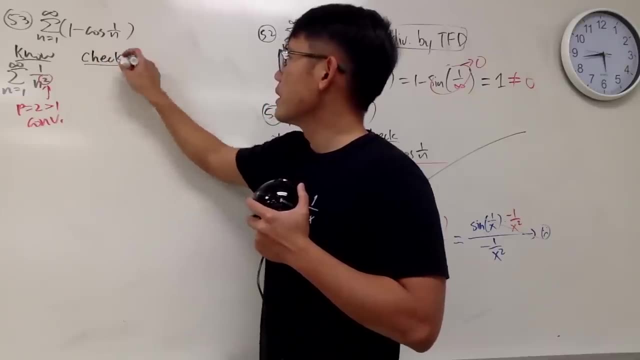 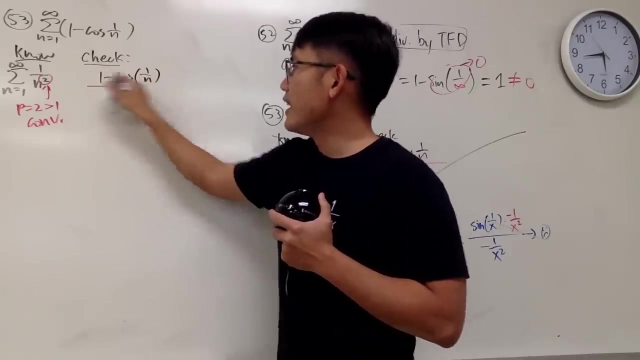 which is greater than 1.. This right here converges. Okay, hope for the best. We'll see Now. check. Okay, here we put this on the top, which is 1 minus cosine of 1 over n and divided by 1 over n, squared. 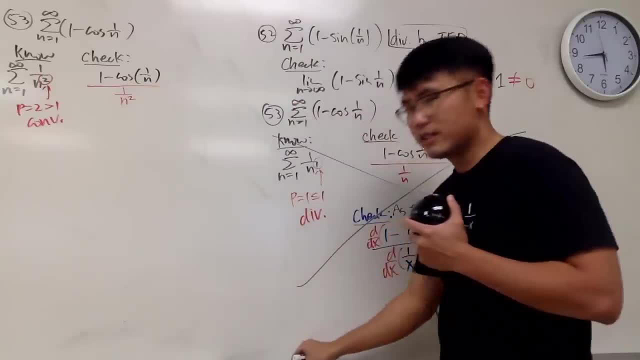 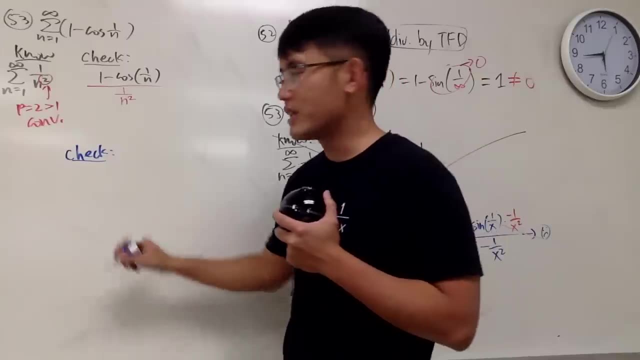 And again we are going to use Laplito's rule. This is a 0 over 0 situation. so we change that to x and do the work. Here we have 1 minus cosine of 1 over x over 1 over x squared. 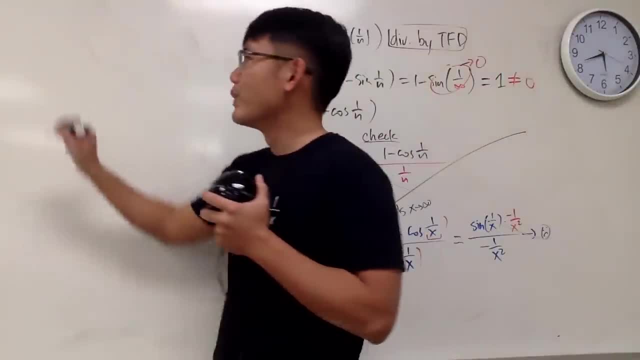 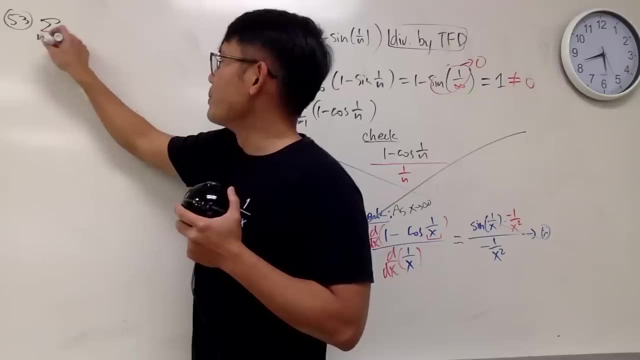 Okay, so this right here didn't work and we just have to do it again, like 53,. just don't give up, And my questions on the exams will be fair enough. so if you just really think about it, if you really prepare, you should be able to do it. 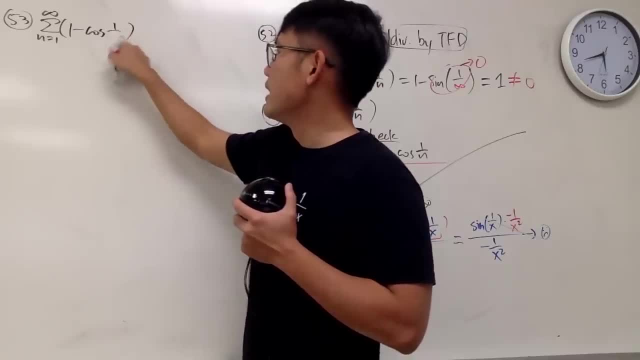 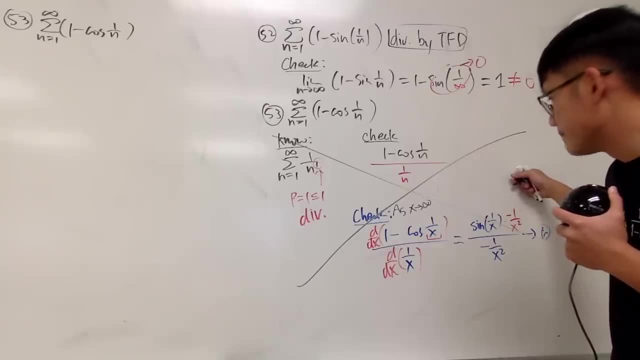 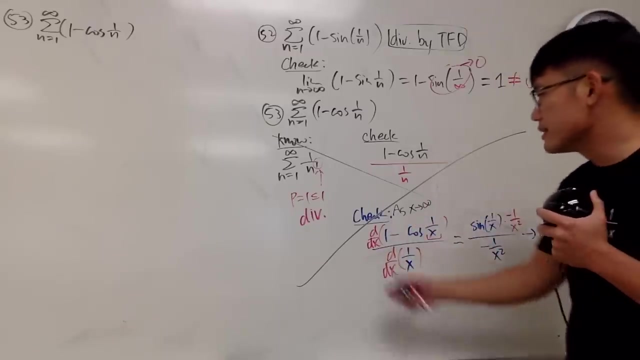 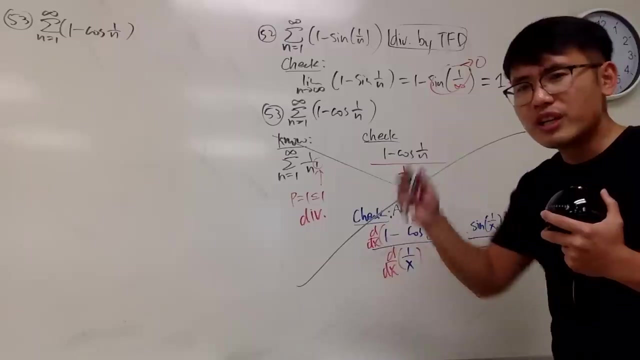 You should be able to handle this kind of things. Oops, not x, it's n right here. Okay, here we go. Seriously, you guys will see why. this doesn't imply anything. okay, Because this right here diverges. and if this is 0, imagine 0 divided by infinity. you can. 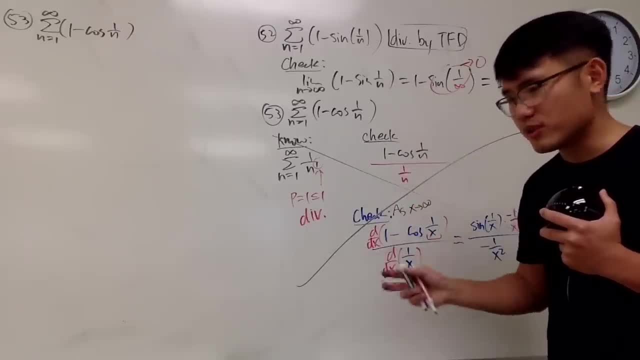 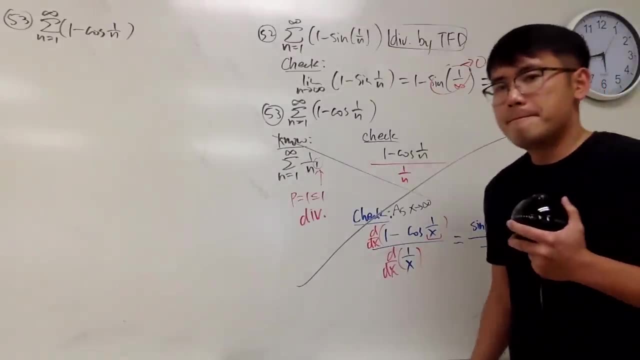 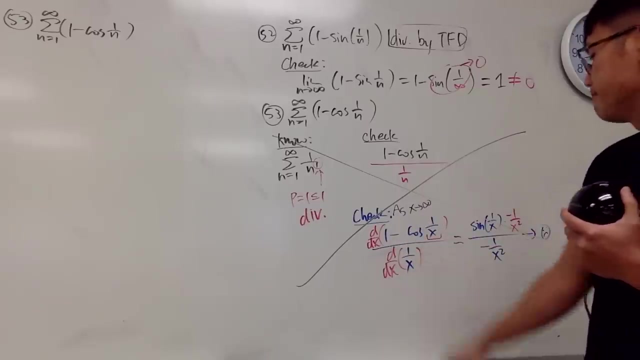 have infinity over infinity still 0, or finite over infinity to be 0, so you cannot really draw a conclusion. That's why 0 is not helping us at all in this case. Hmm, Maybe it converges because, again, if you do this, divided by that, that was a divergent. 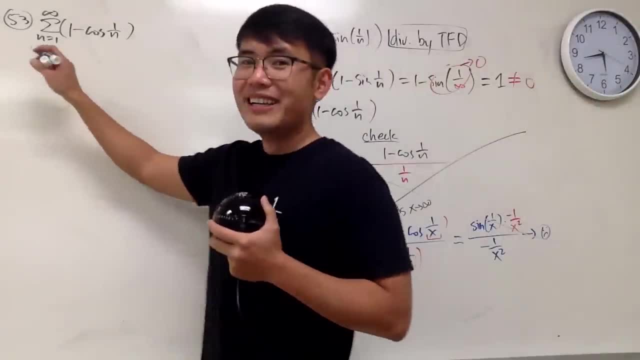 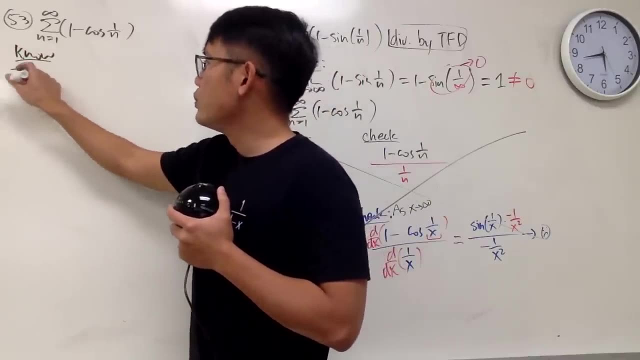 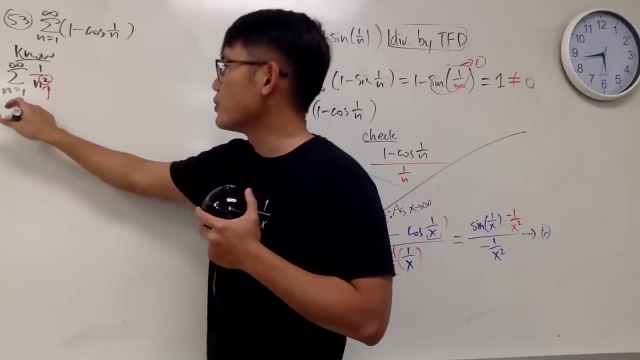 So let me try the other one. Let me try. Let me try the other one. So suppose we do the following. Suppose I want to use the sum as n goes from 1 to infinity of 1 over n squared. Let me try the convergent version, which is: p is 2, which is greater than 1.. 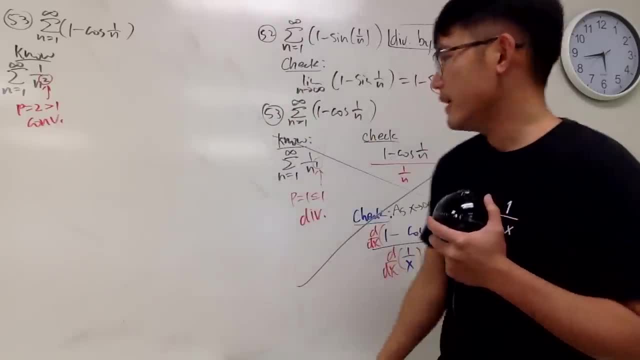 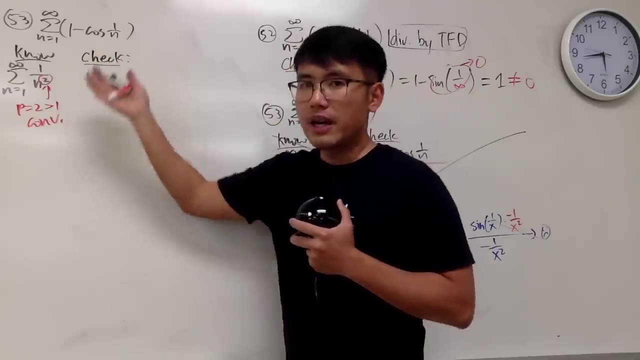 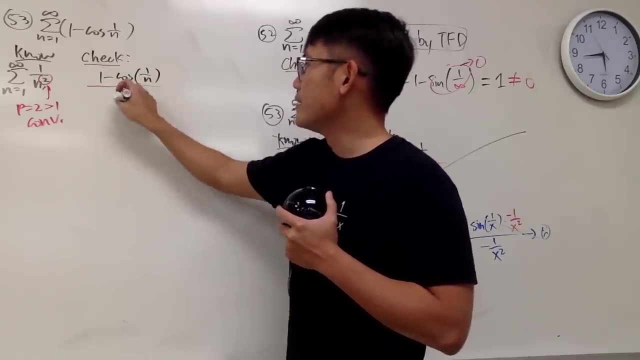 This right here converges. Okay, Hope for the best. We'll see Now check. Okay, here we put this on the top, which is 1 minus cosine of 1 over n and divided by 1 over n squared. 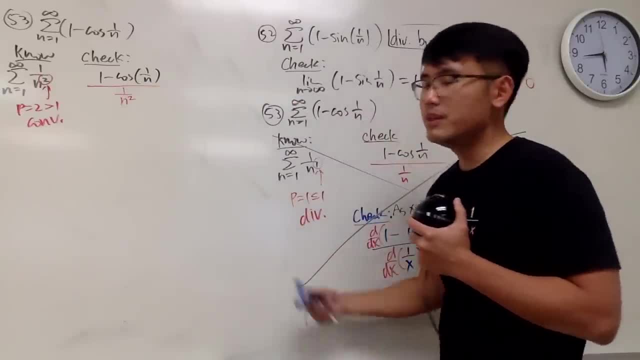 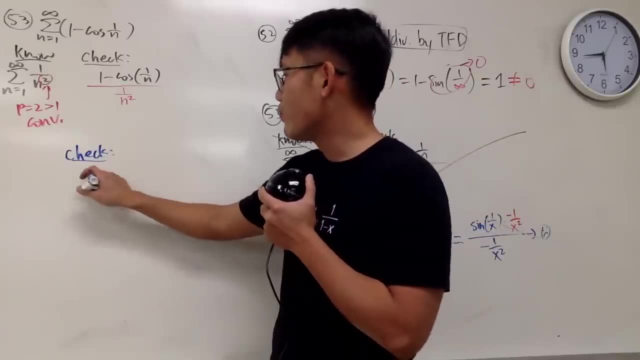 And again we are going to use Laplito's rule. This is 0 over 0.. 0 over 0.. See true Asian. So we change that to x and do the work. Here we have 1 minus cosine of 1 over x over, 1 over x squared. 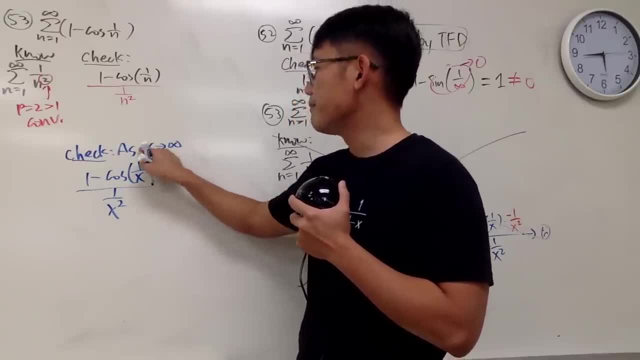 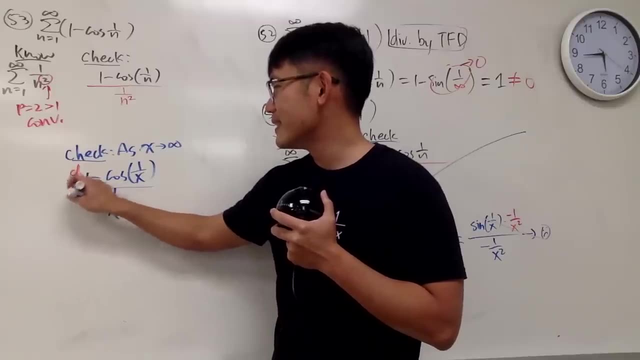 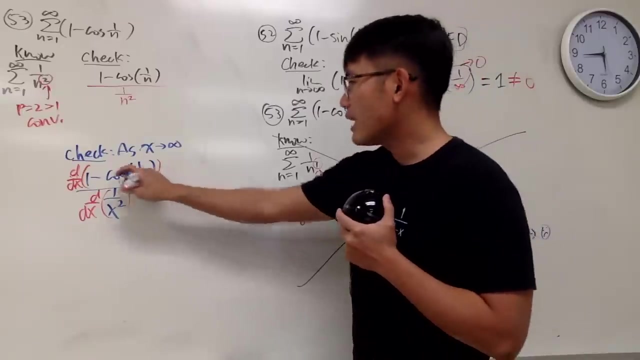 And this is again as x going to infinity. Now take the derivative of the top and also the derivative on the bottom. Hmm, On the top, this right here we get positive sign. Oh, We get a negative sign here. 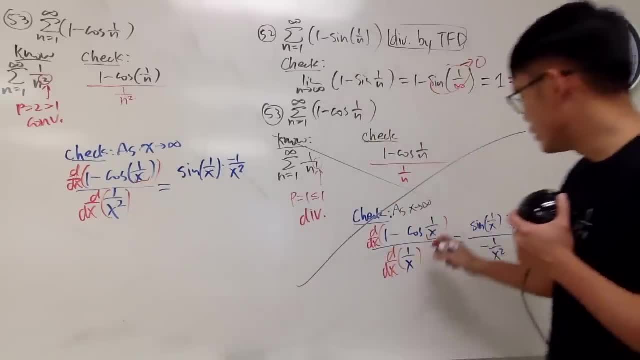 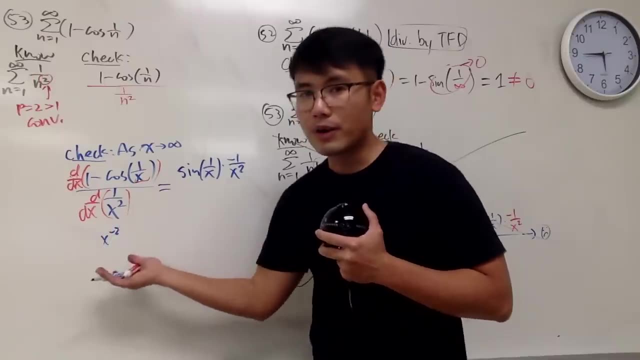 So this is negative sign. So we take the derivative of 1 over x and multiply by negative 1 over x. squared Right Again, chandelier. don't forget about the chandelier right here. Okay, Now for the bottom. here this is: I say x to the second. well, negative 2 power like 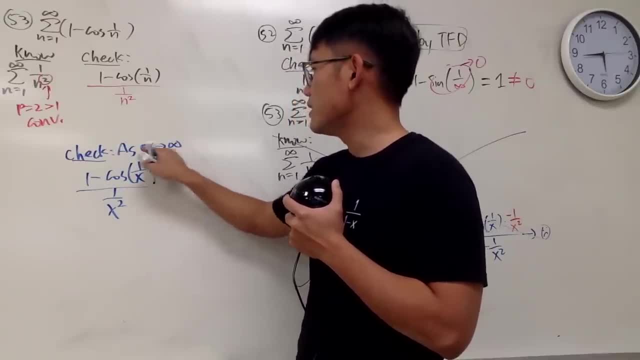 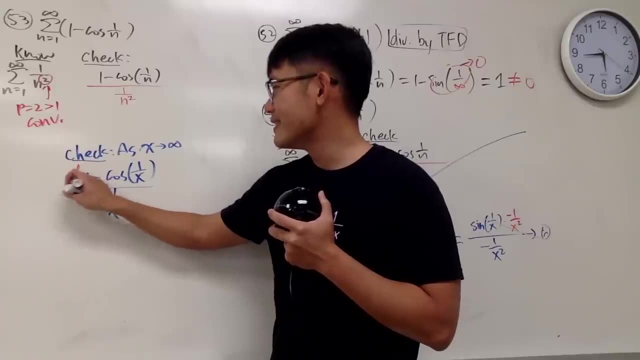 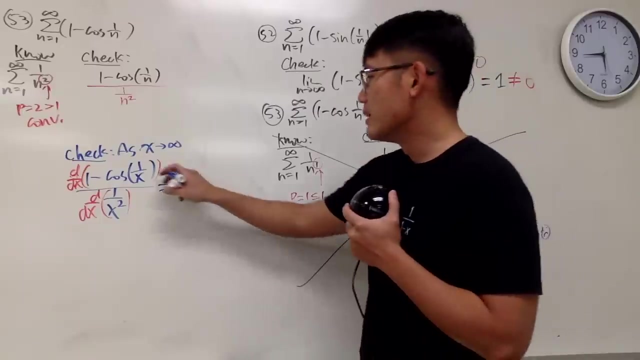 and this is again as x going to infinity. Now take the derivative of the top and also the derivative on the bottom. On the top, this right here, we get positive sign of 1 over x and multiply by negative 1 over x, squared. 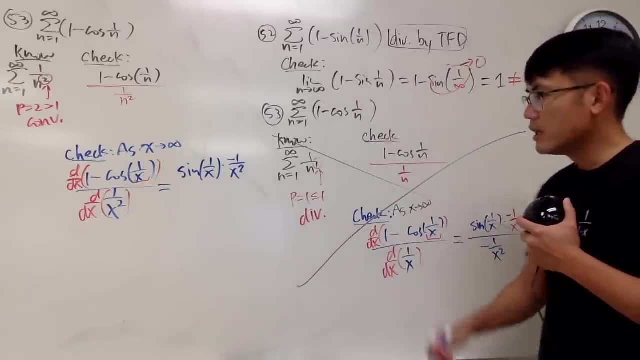 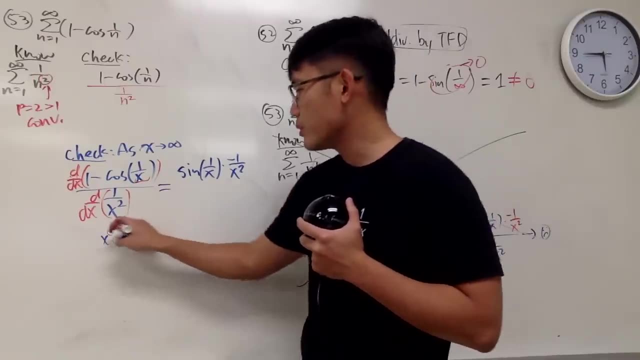 Again, Chengdu. Don't forget about the Chengdu right here. Now for the bottom. here this is: I say x to the second, well, negative 2 power like this. So bring the power to the front and the minus 1.. 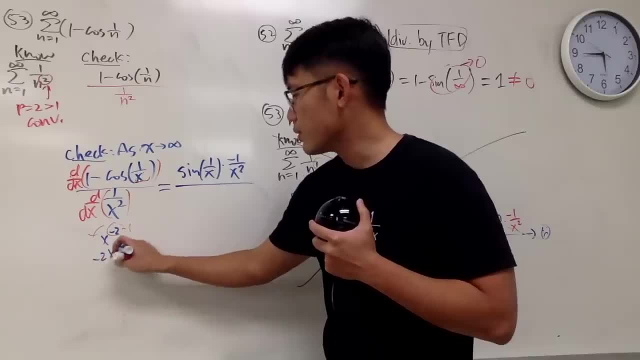 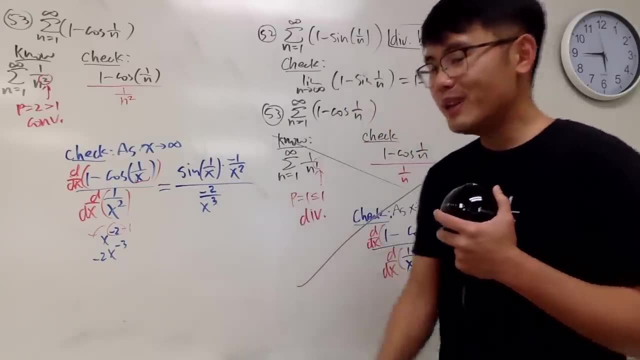 So we have to divide it by negative 2, x to the negative 3,, which is negative 2 over x to the third, Like this. okay, Now here is the simplification: We will multiply the top and bottom by x to the third power. 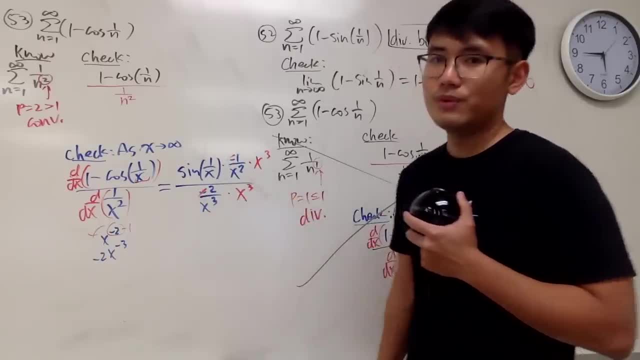 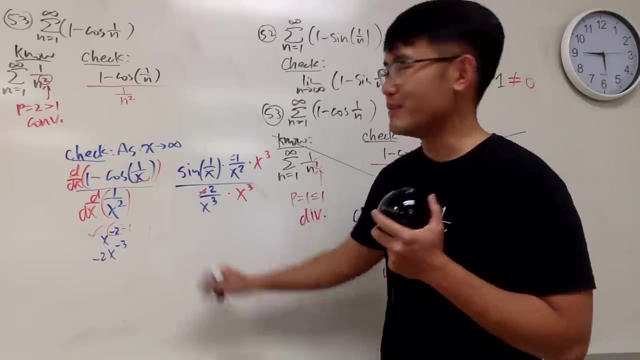 And we can also get rid of the negative signs. Why not Now? we see, technically I should draw the arrow because we have to take the limit, Because this to this is because of Laplito's rule. So, from here to here. 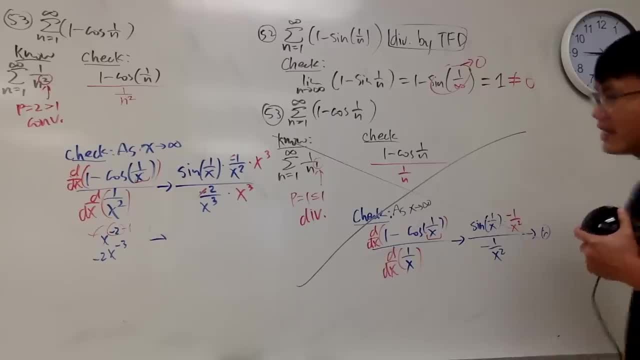 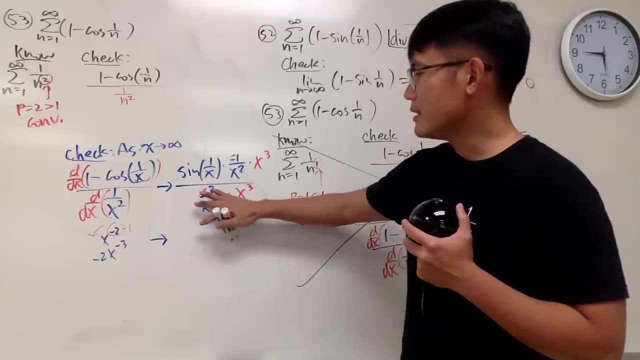 I should technically draw an arrow, But yeah anyway. Okay, Now on the top. well, on the bottom, this is gone. We have the 2 on the bottom, So I'll put down the 1 half here. 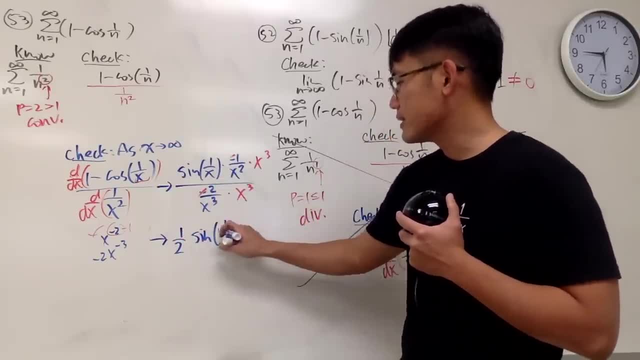 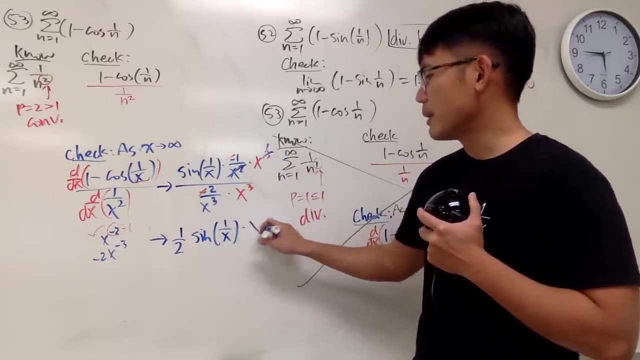 And we see that we have sine of 1 over x And this and that you can see this and that cancel. We have 1 left, So it's multiplied by x. Check this out. We have an x right here. 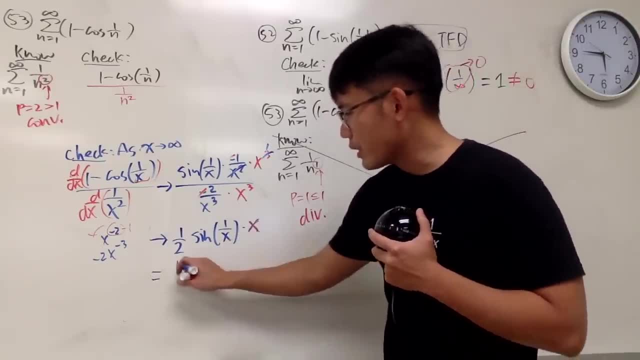 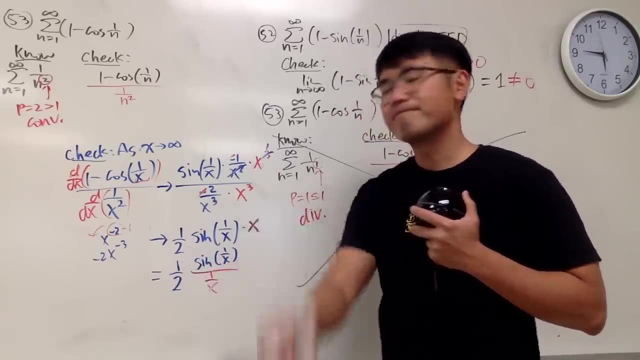 We can bring this down again. So this right here is equal to- because I'm doing algebra times- sine of 1 over x over 1 over x, When x is going to infinity. this and that are the same And they are both approaching 0.. 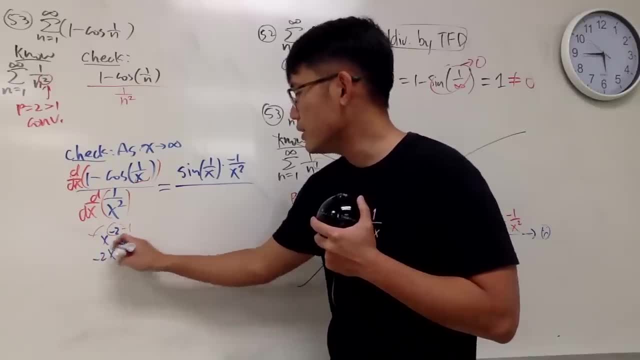 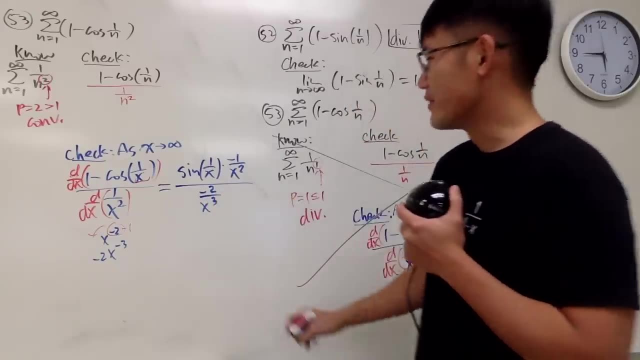 this. So I bring the power to the front and a minus 1.. So we have to divide it by negative 2x to a negative 3, which is negative 2 over x to the third power, like this: Okay. 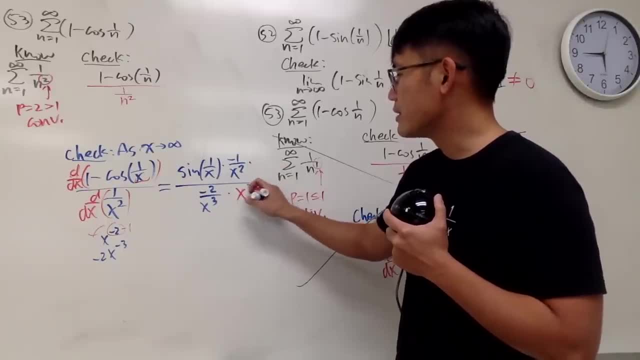 Now here is the simplification: We will multiply the top and bottom. Okay, So we have negative 2x to a negative 3, which is negative 2 over x to the third power. like this: Okay, the top and bottom by x to the third power. 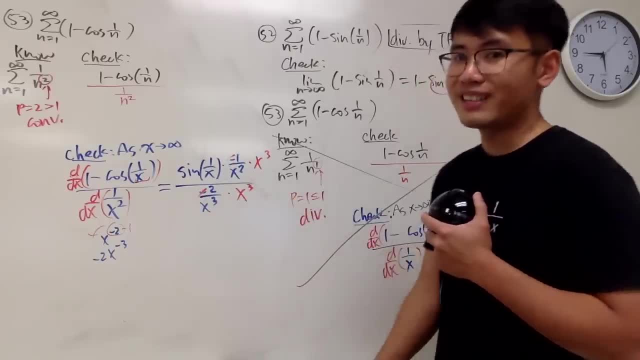 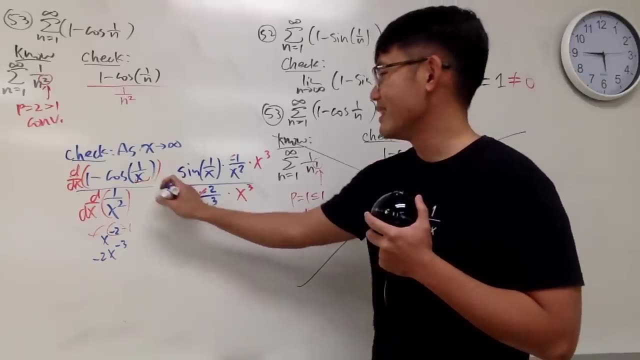 And we can also get rid of the negative signs. Why not Now? we see, technically I should draw the arrow because we have to take the limit, Because this to this is because of Lapito's rule. So, from here to here, 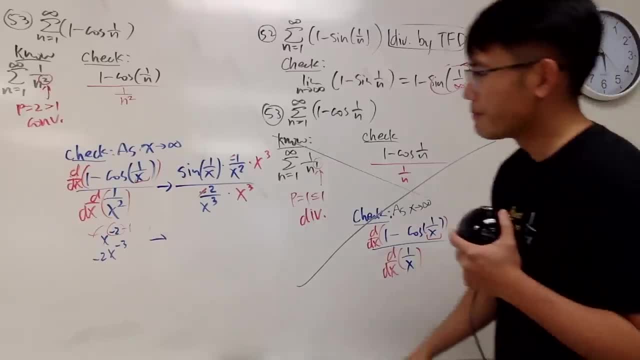 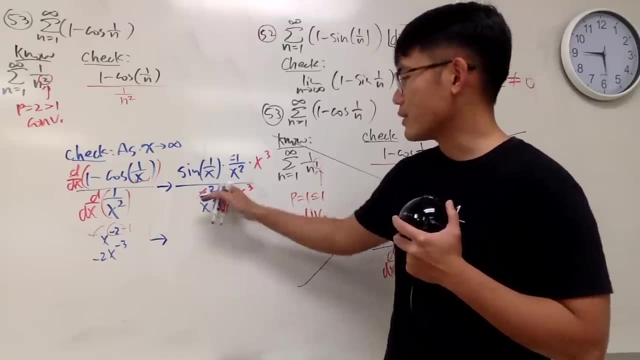 I should technically draw an arrow, But yeah anyway. Okay now on the top. well, on the bottom, this is gone. We have the 2 on the bottom, so I'll put down the 1 half here. 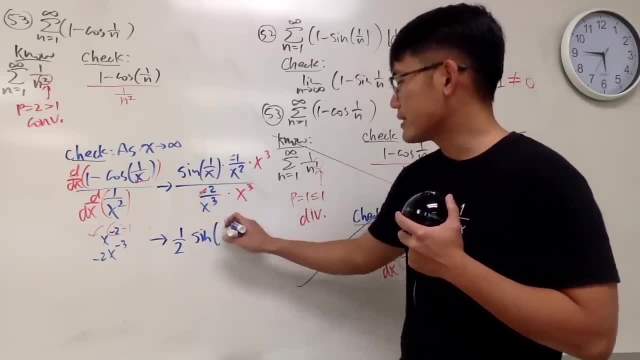 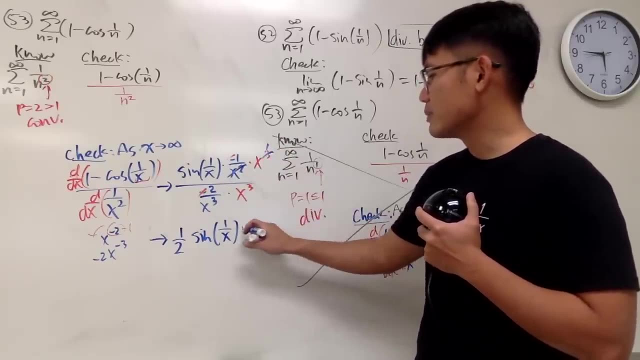 And we see that we have sine of 1 over x And this and that you can see this and that cancel. We have 1 left, So it's multiple by x. Check this out. We have an x right here. 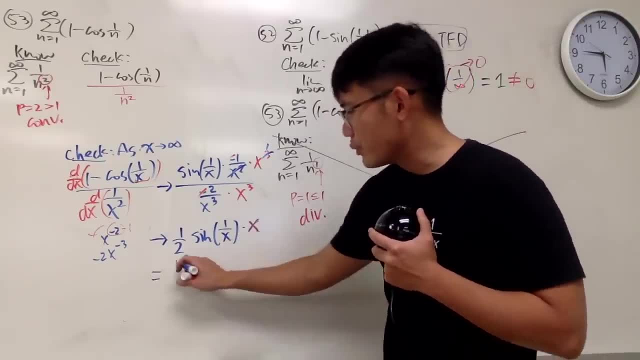 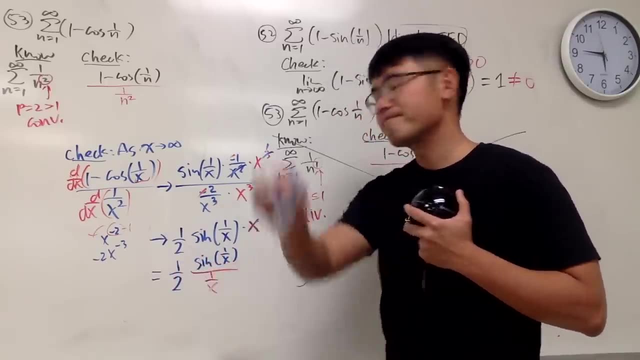 We can bring this down again. So this right here is equal to- because I'm doing algebra- 1 half times sine of 1 over x over 1 over x. Okay, So when x is going to infinity, this and that are the same. 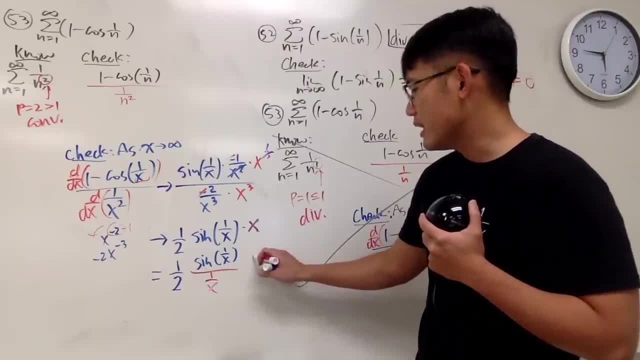 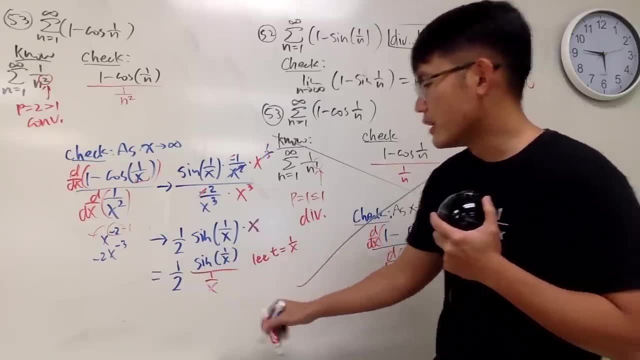 and they are both approaching 0.. You guys know the deal. If you would like, you can say that. well, t equal to 1 over x. So this right here will actually going to be like sine t over t, So this is 1 over 2. 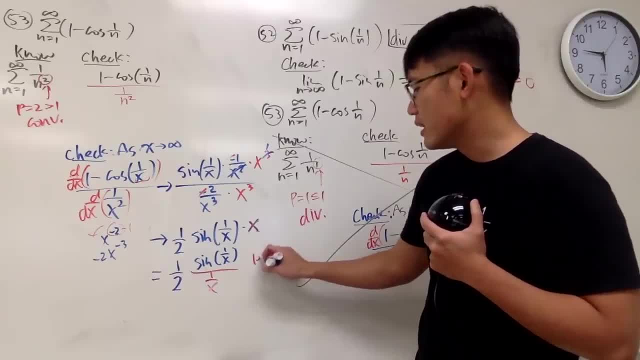 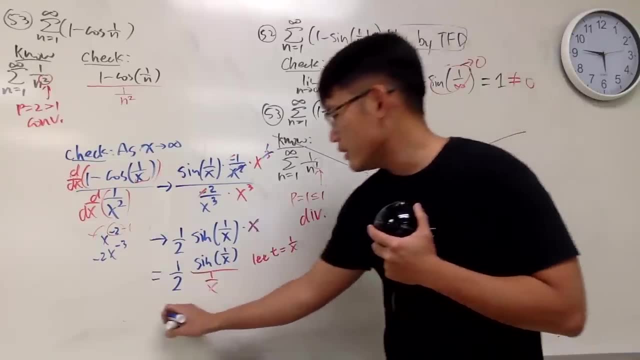 You guys know the deal. If you would like, you can say that: well, t equal to 1 over x. So this right here is actually going to be like sine t over t. So this is 1 over 2. 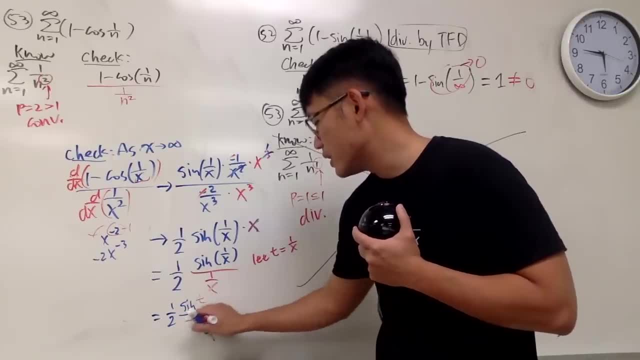 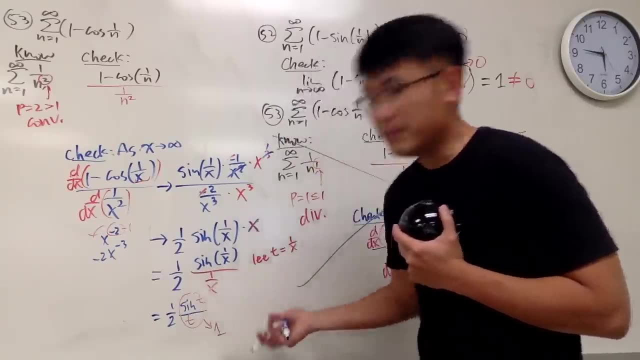 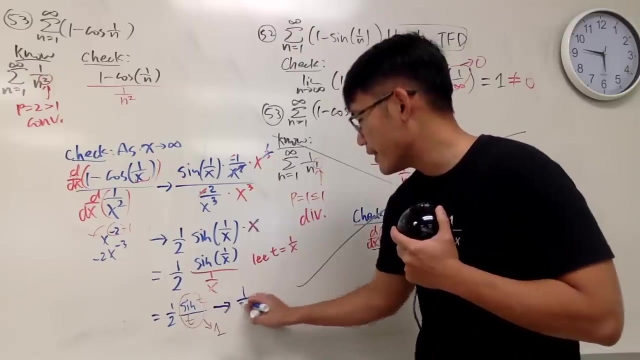 sine t over t. But anyway, the truth is I chose this approach. 1. Because, thank god, the limit right. So, all in all, this right here approaches this, right here approaches 1 half like this: 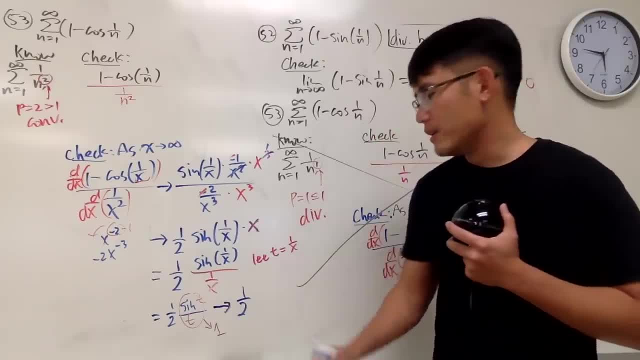 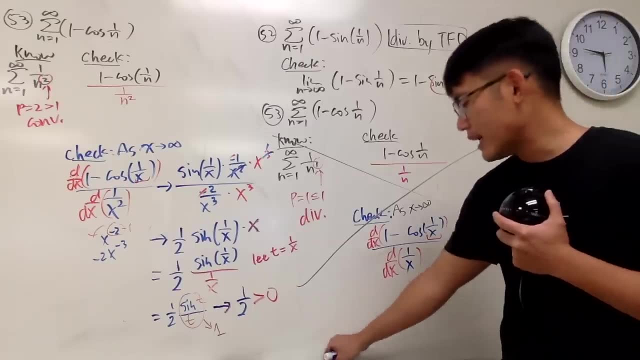 And because this is positive- 1 half- it's useful. 1 half is greater than 0.. The limit comparison test is useful in our case And of course I also have to show you guys that if the function version has a limit- 1 half- 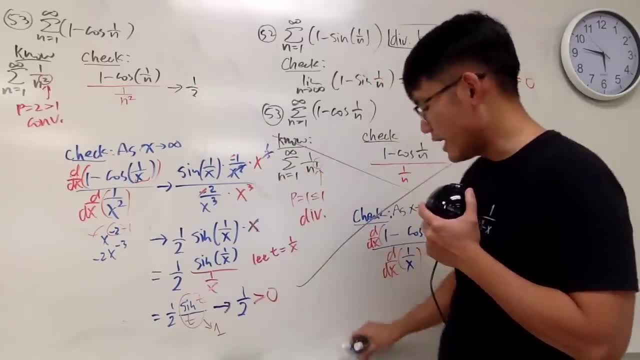 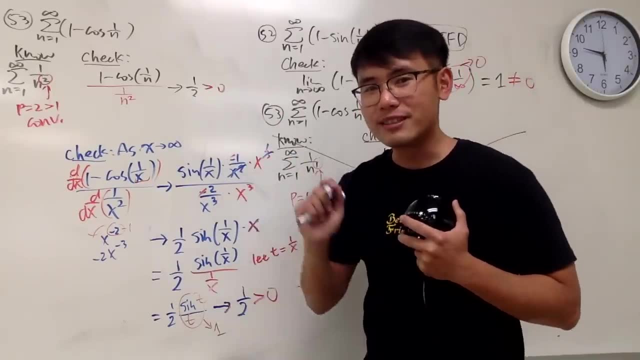 this right here- also approaches 0. This 1 half- which we can also say this right here- is greater than 0. This is useful in the limit comparison test And they have the same conclusion. So therefore I will come back here and say: 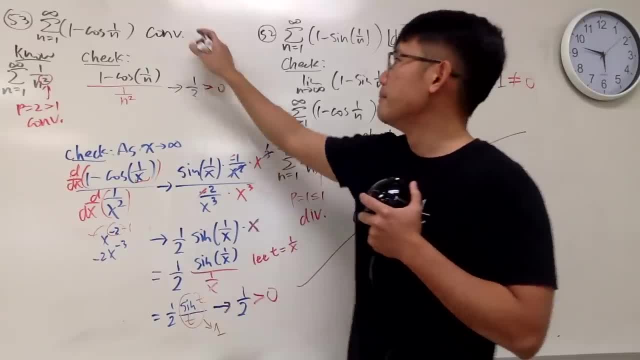 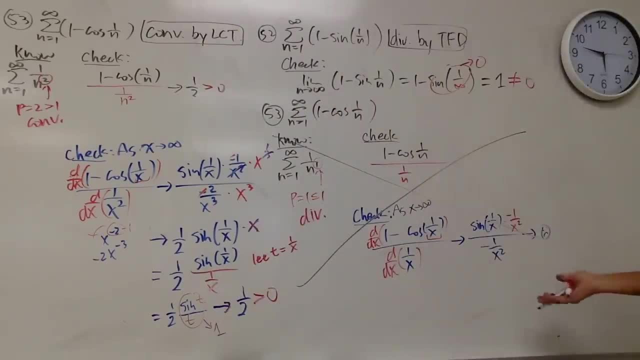 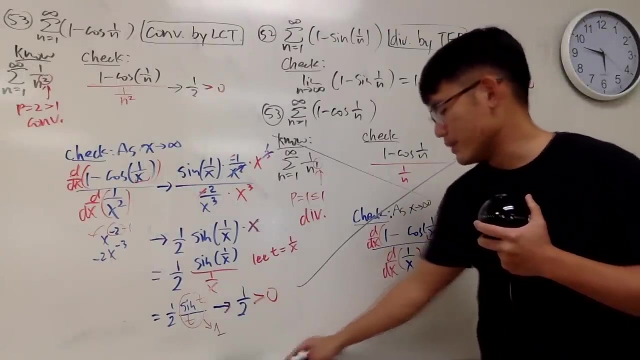 this right here actually converges by the limit comparison test And we are done. So again, be really careful with this. This is actually one of the harder questions I will say Right. So again, if necessary, I will just give you guys. 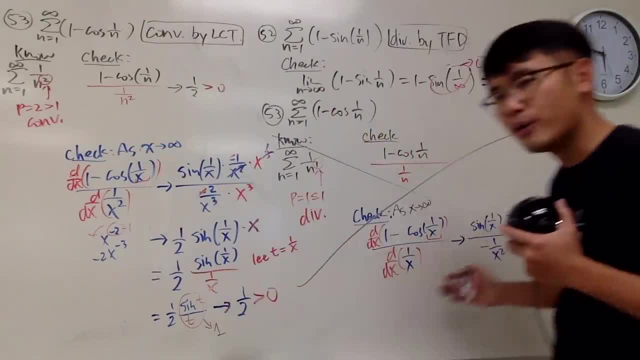 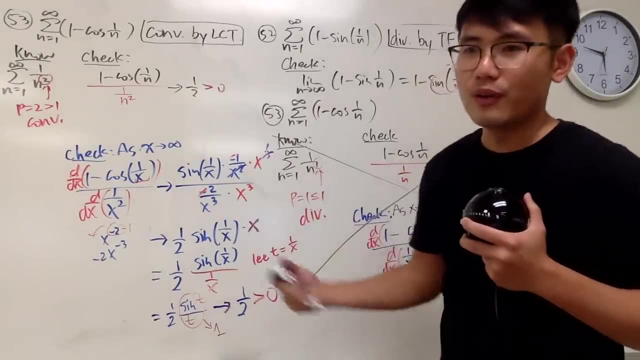 consider to compare with this or that, And you have to know this right here. we have to. we can natural conclusion: just have to erase this and then redo the whole thing. Hopefully we will get it right. That's the idea. 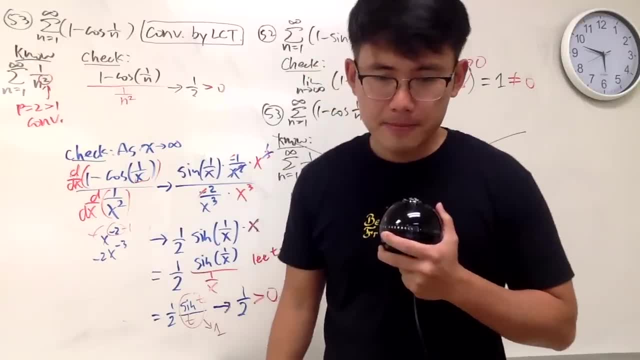 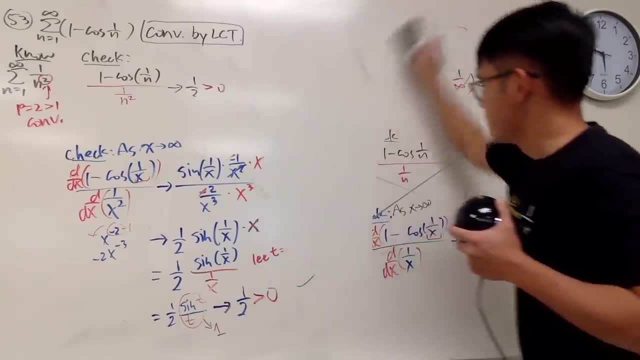 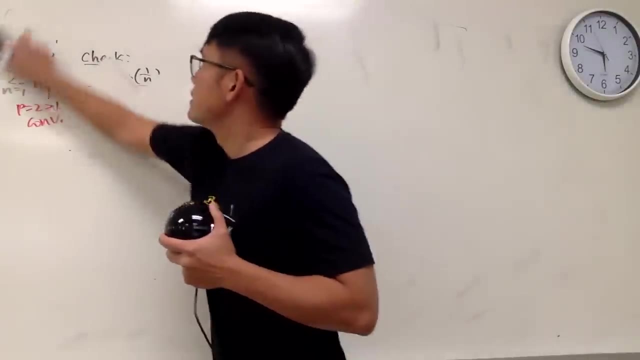 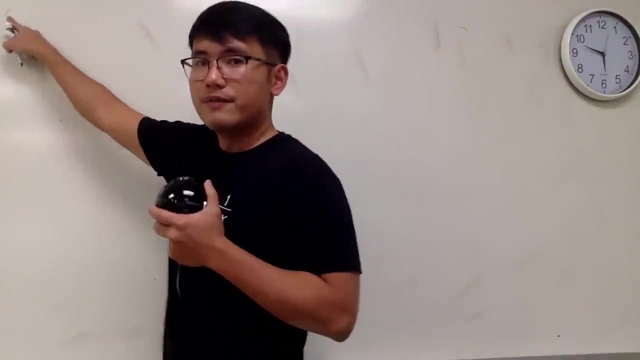 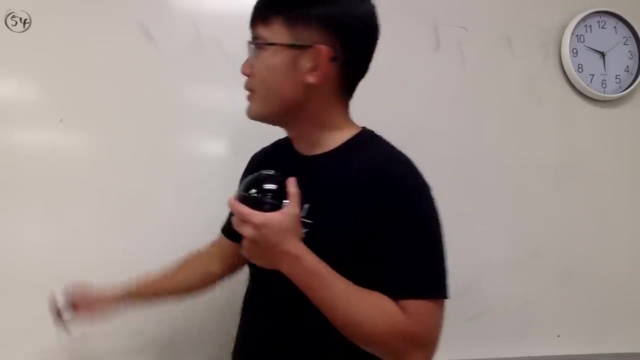 Hmm, Okay, All right, Now let's do the other ones. Number 54.. Right here, Number 54.. Number 54. We have to have the sum, as n goes from 1 to infinity And we have 1 over. 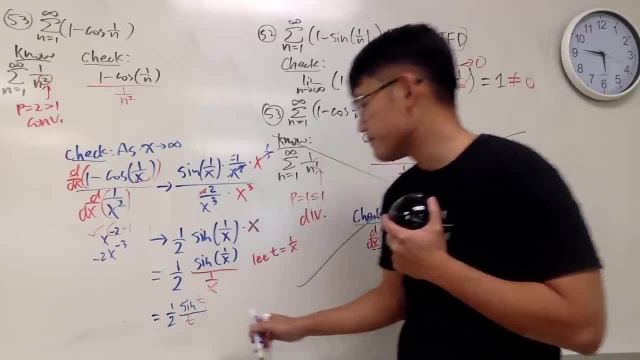 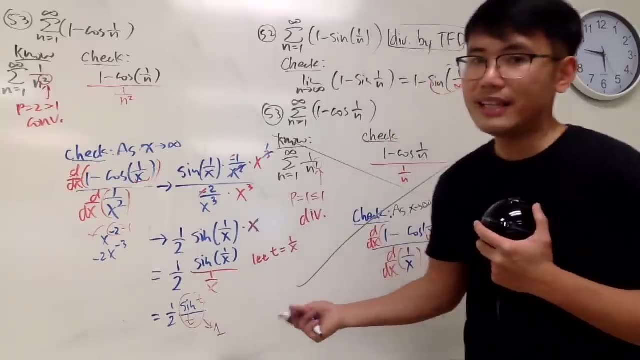 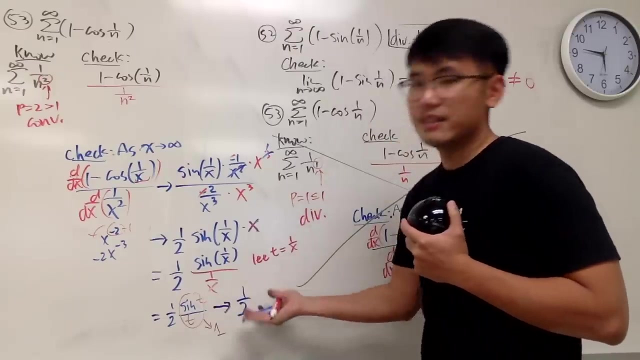 sine t over t. But anyway, the truth is I chose this approach 1. Because, thank God, the limit right. So all in all this right here approach, this right here approach 1, half like this: 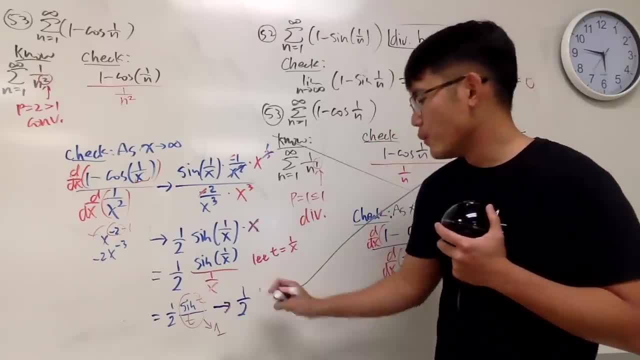 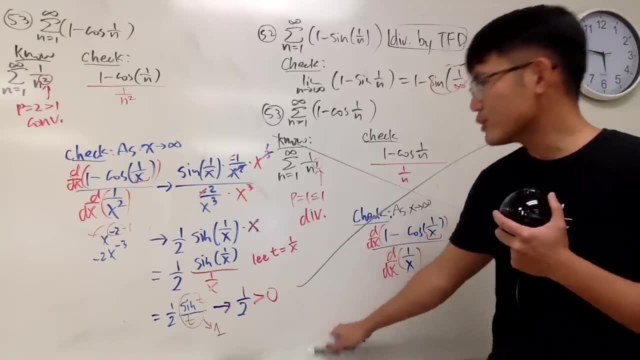 And because this is positive- 1 half- it's useful. 1 half is greater than 0.. The limit comparison test is useful in our case And of course I also have to show you guys that if the function version has a limit- 1 half- 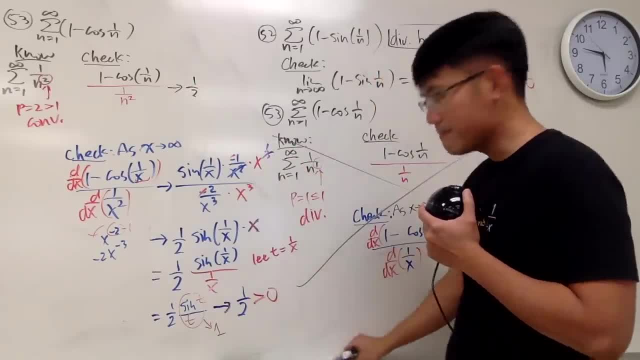 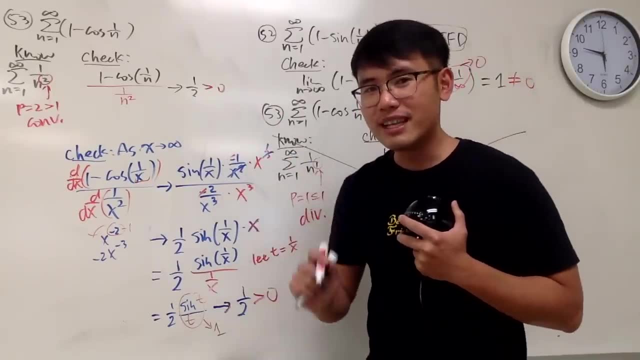 this right here also approaches 1 half, which we can also say this right here- is greater than 0. This is useful in the limit comparison test, This is useful in the limit comparison test And they have the same conclusion. So therefore, I will come back here and say: 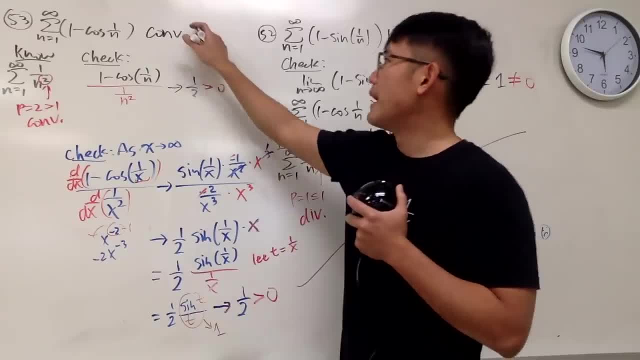 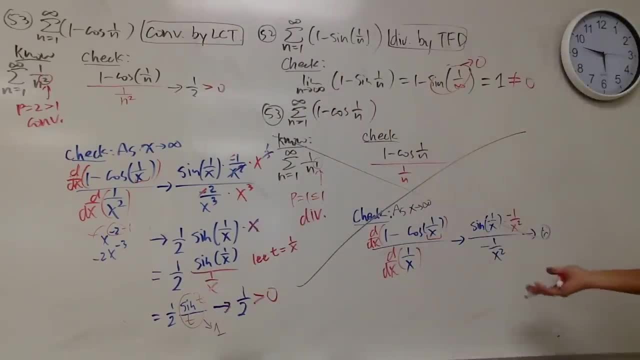 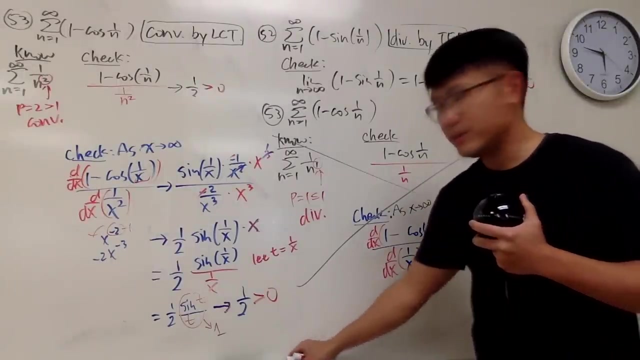 this right here actually converges by the limit comparison test And we are done. So again, be really careful with this. This is actually one of the harder questions. I will say Right And again, if necessary, I will just give you guys. 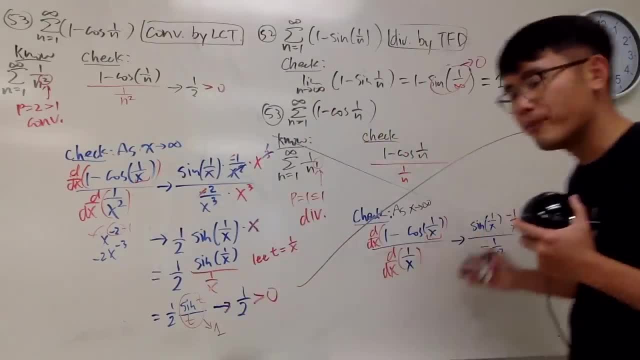 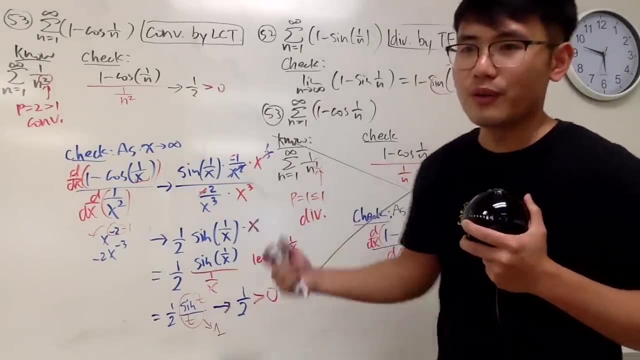 consider to compare with this or that, And you have to know this right here. We have to. we will connect your conclusion. Just have to erase this and then redo the whole thing. Hopefully we will get it right. That's the idea. 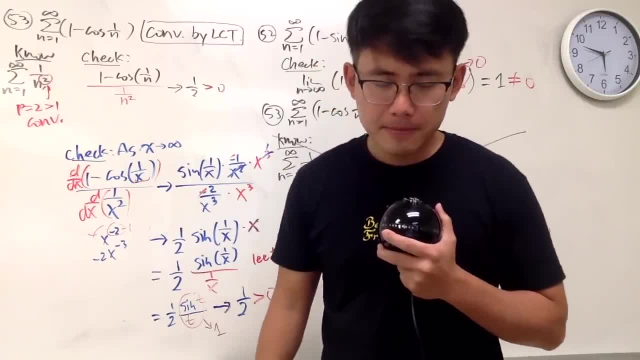 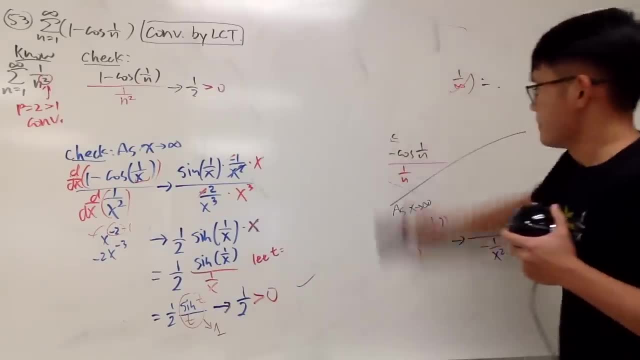 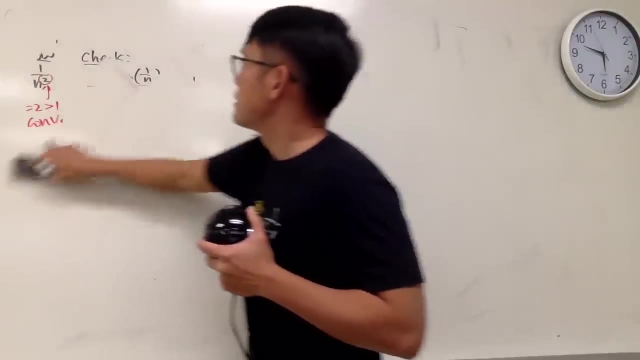 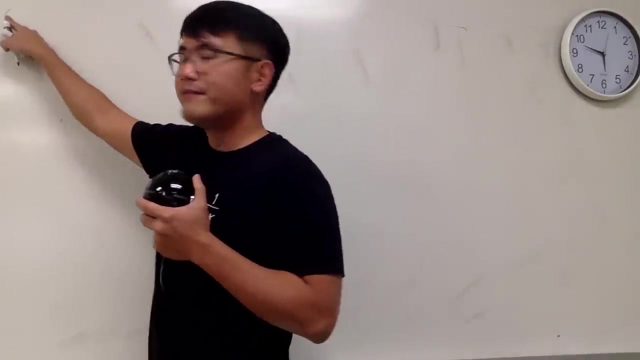 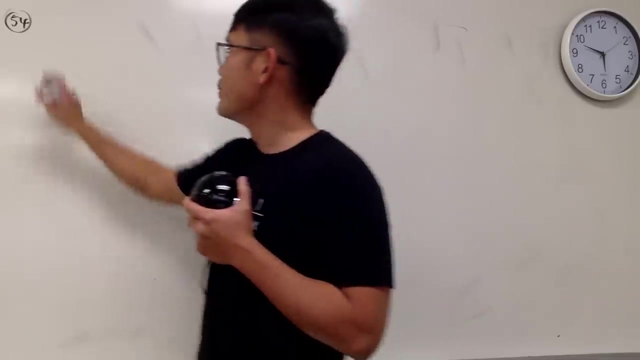 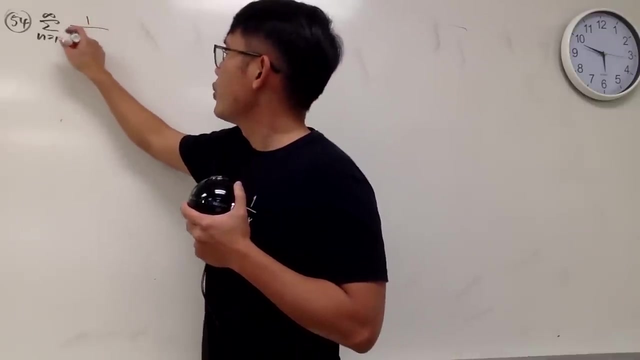 Hmm, Okay, All right, now let's do the other ones. Number 54, right here, Number 54,, number 54. We have to have the sum as n goes from 1 to infinity And we have 1 over the cube root of 2 to the n plus 1, like this: 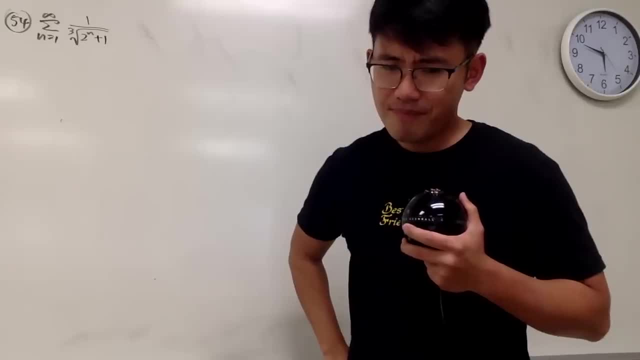 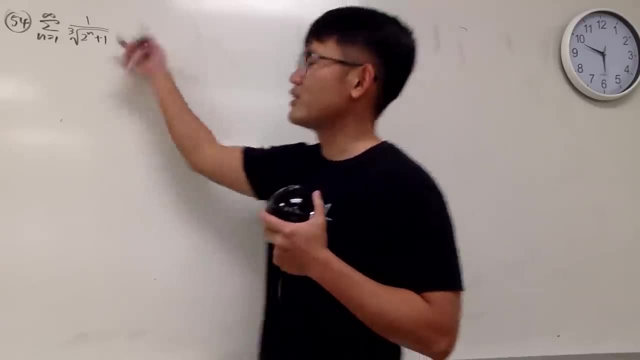 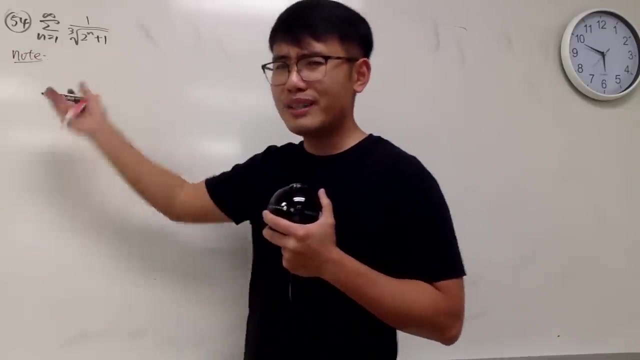 Okay, Hmm, Okay, Why not? let's just take out the 1.. The 1 is bothering us, huh. So notice the following: We can just take out the 1. And you see the 2 to the n, so it has a good chance to be a convergent right. 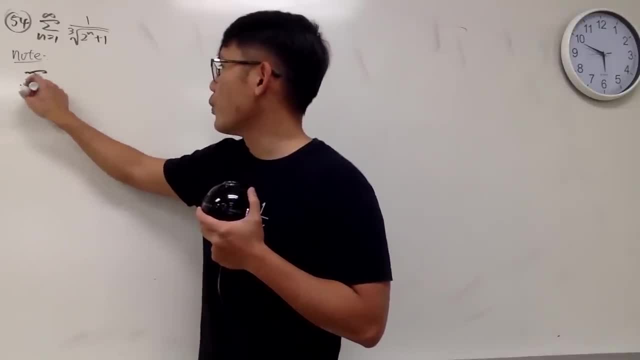 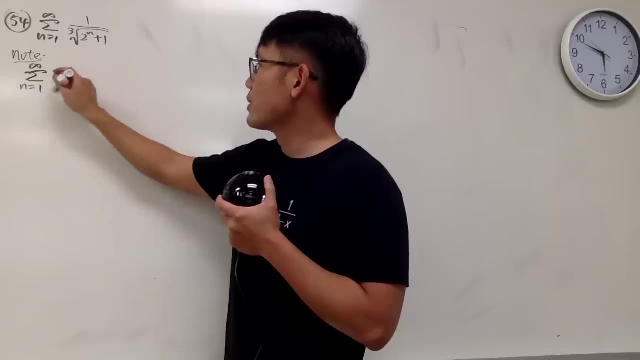 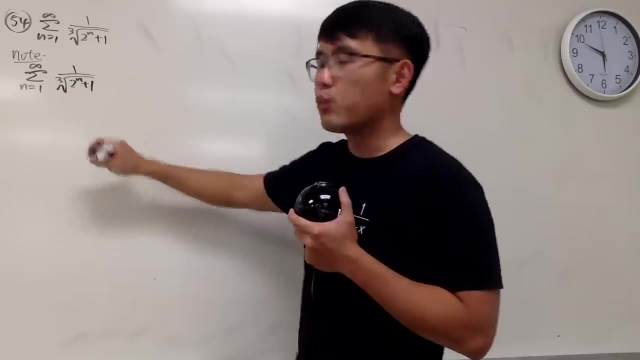 So we just have to do the computation to make sure that all the work, all the inequalities, works out nicely. So now look at the sum: as 1 goes to, as n goes from 1 to infinity. This right here, the moment we remove the plus 1,. 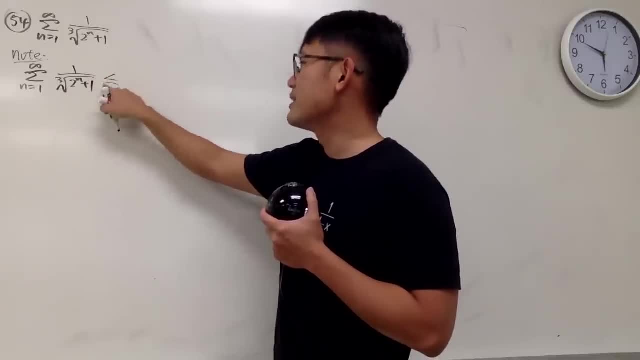 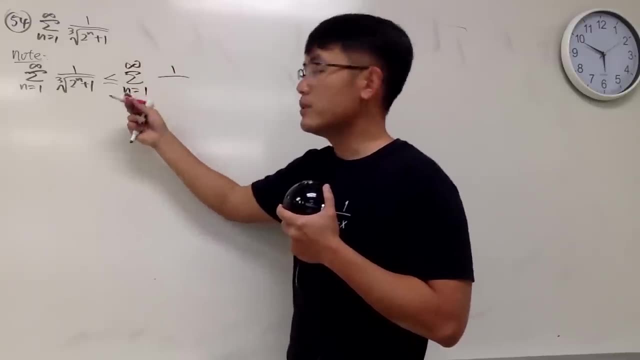 it will be less than or equal to, technically less than. but if I have to be more serious, And this right here goes from 1 to infinity and we have just 1 over the cube root of the, let's just do it this way. this is the cube root. 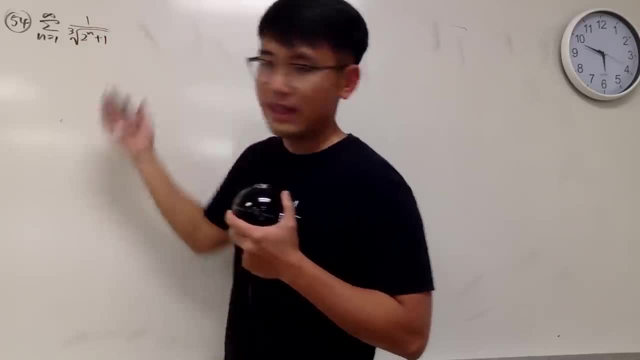 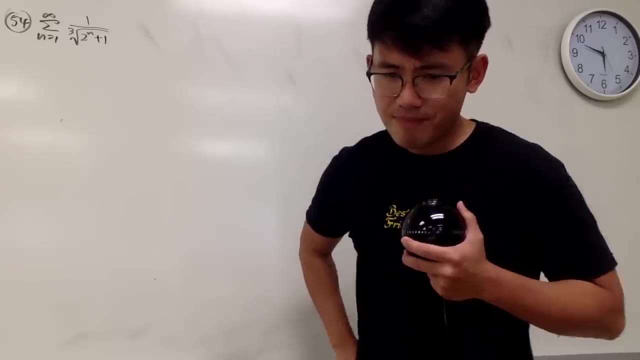 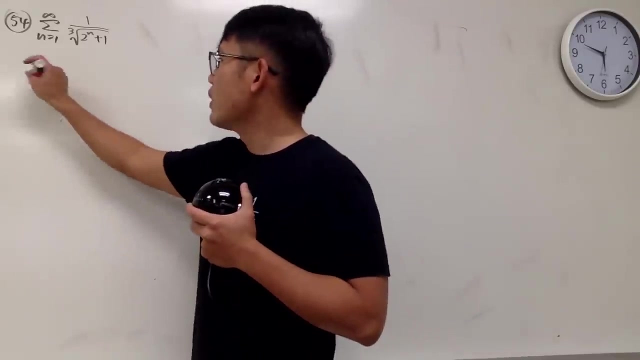 the cube root of 2 to the n 1 like this: Okay, Hmm, Okay, Why not? Let's just take out the 1.. The 1 is bothering us, huh. So notice the following: We can just take out the 1.. 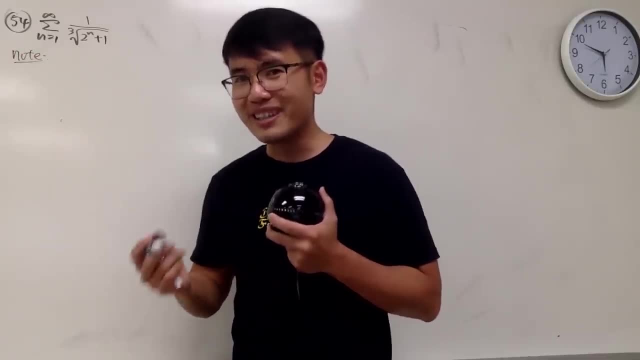 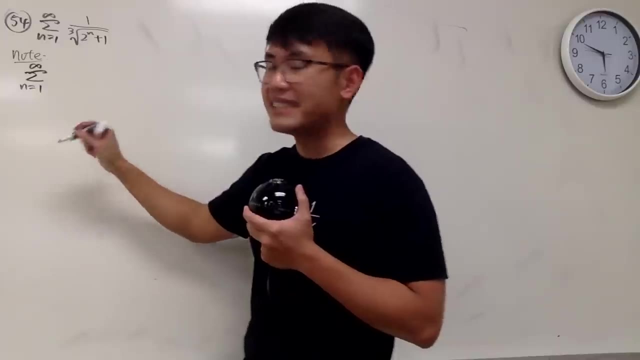 And you see the 2 to the n. So it has a good chance to be a convergent right. So we just have to do the computation to make sure that all the work, all the inequalities, works out nicely. So now look at the sum. 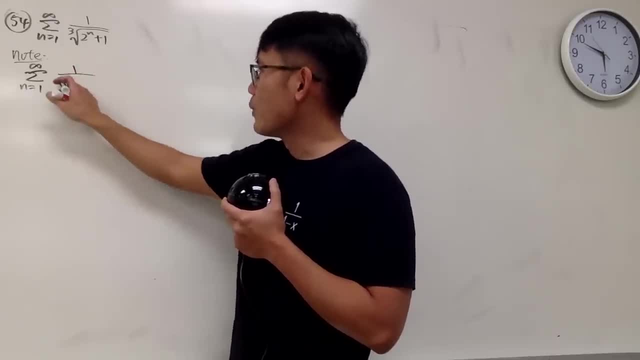 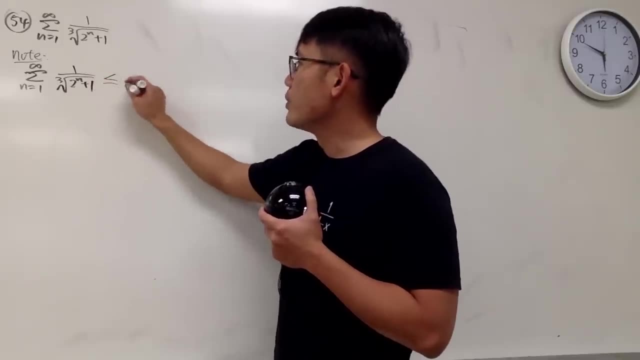 as 1 goes to 1 goes, as n goes from 1 to infinity. This right here, the moment we remove the plus 1, it will be less than or equal to, technically less than by the 5, seriously, 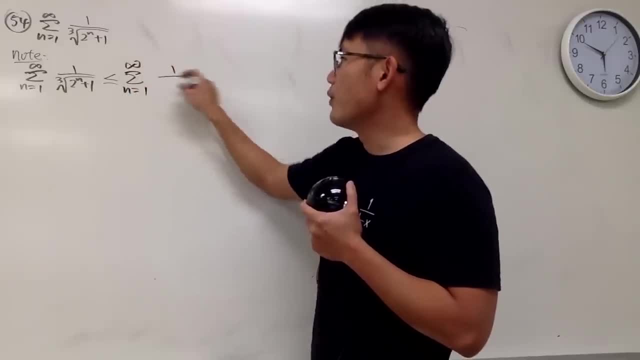 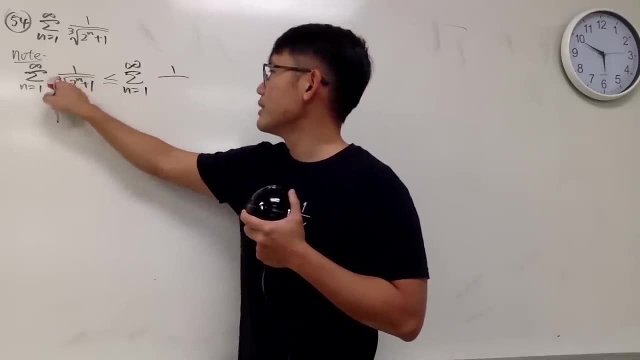 And this right here goes from 1 to infinity and we have just 1 over the cube root of the. let's just do it this way: This is the cube root. ah, this is the cube root, right, And let me just write this down first. 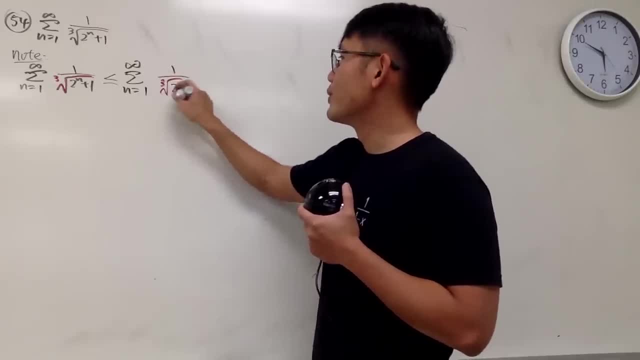 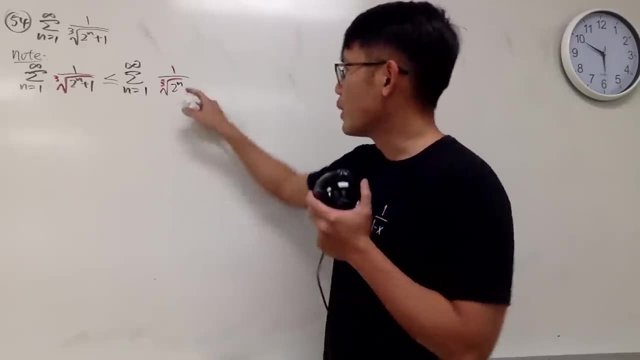 Let me just write down: this is the cube root of 2 to the n, like that. And now here is the DO. Don't forget this is the same as 1 third power. So we have 2 to the n to the 1 third power. 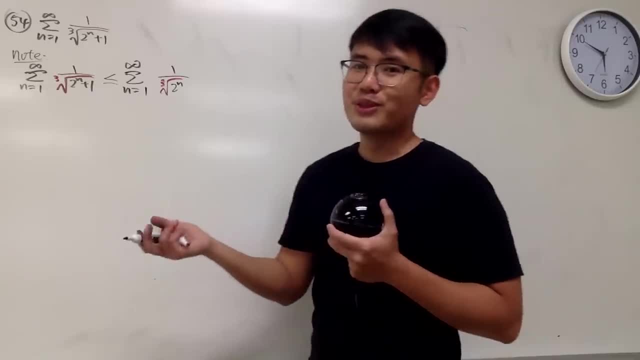 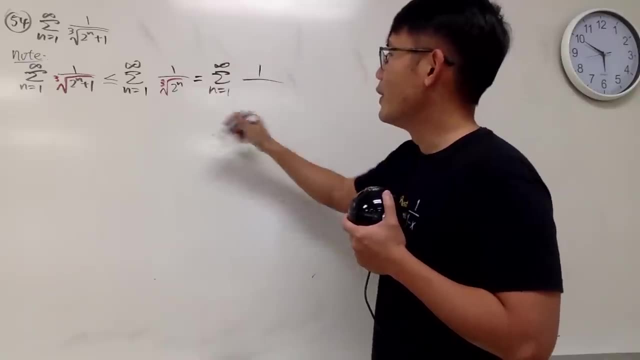 So in another word: oh, you can also just do this if you would like This right here, it's actually equal to the sum, as n goes from 1 to infinity 1 over. we can do the cube root first. 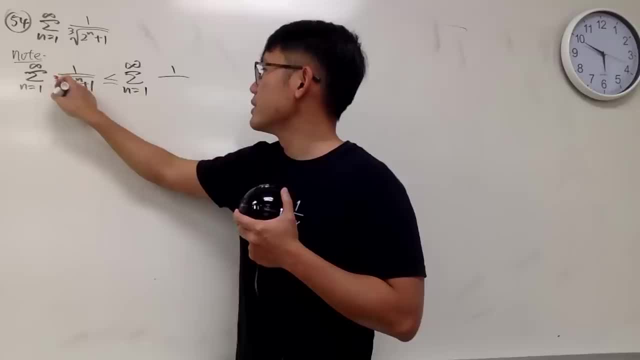 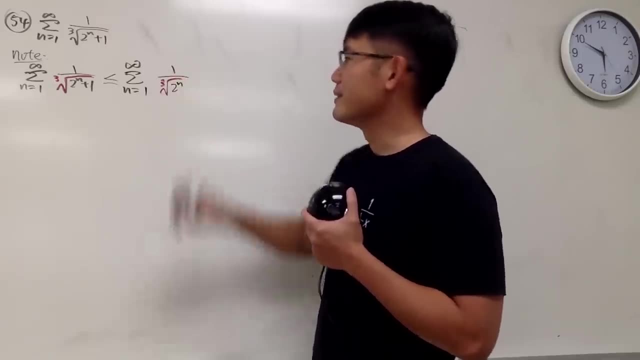 this is the cube root, right, And let me just write this down first. Let me just write down: this is the cube root of 2 to the n, like that. And now here is the DO. Okay, Don't forget, this is the same as 1, 3rd power. 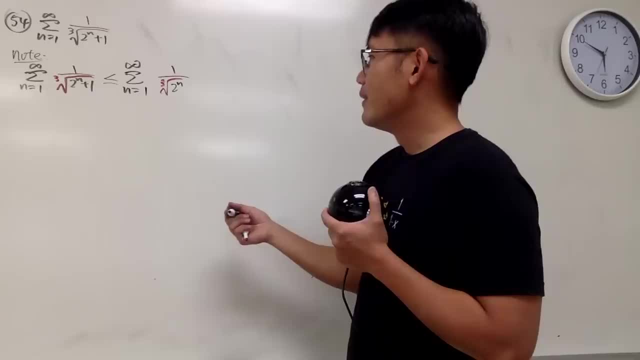 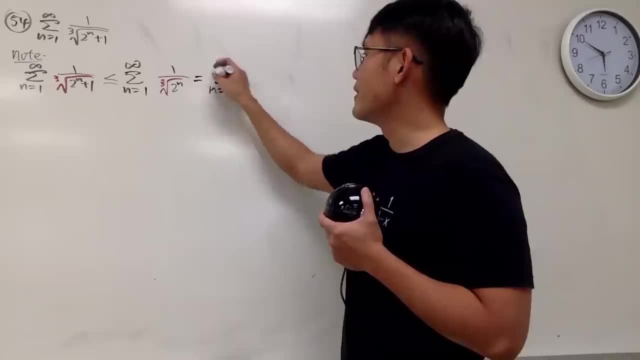 So we have 2 to the n to the 1 3rd power. So in another word- or you can also just do this if you would like This right here- is actually equal to the sum as n goes from 1 to infinity, 1 over. 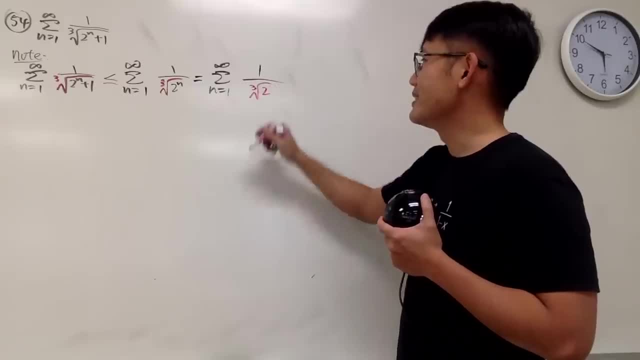 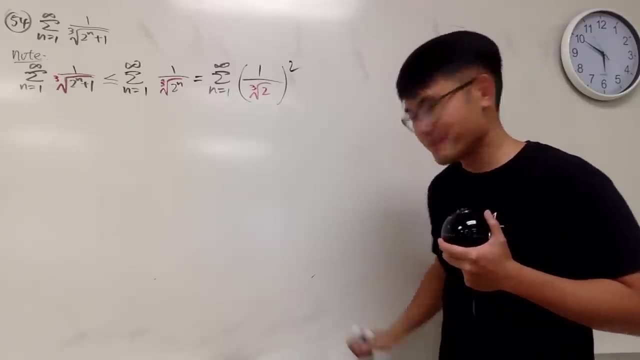 we can do the cube root first Cube root of 2, like this, And then the nth power, And then we can just put the nth power on our side, Like that. Very nice, huh. And now we are doing two things. 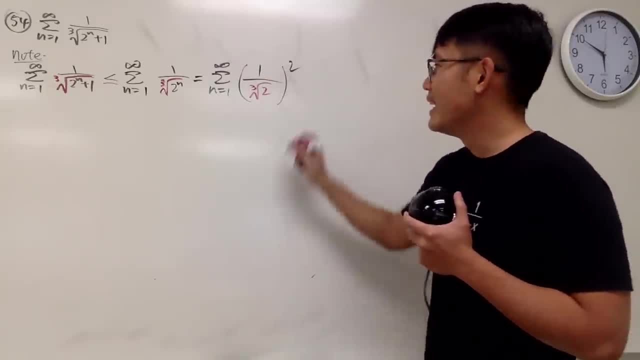 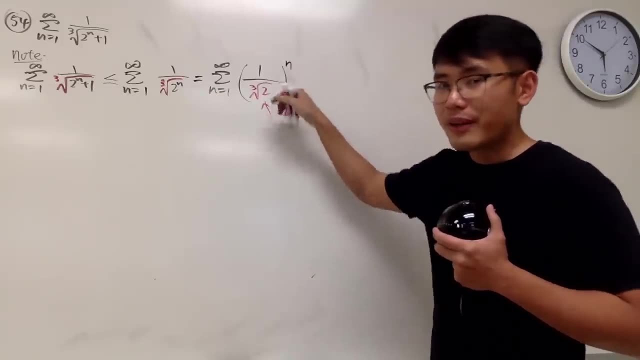 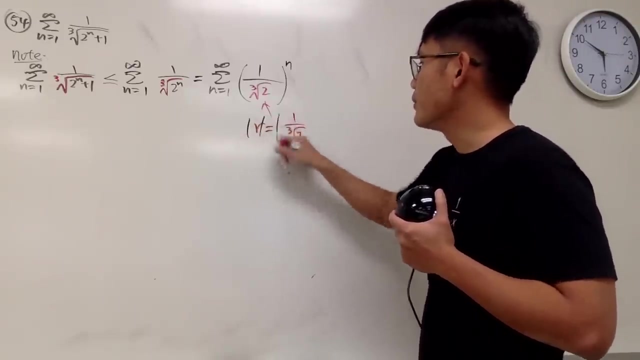 As you can see, this right here is what This right here is actually. oops, not 2.. n This right here is the common ratio r, which is 1 over the cube root of 2.. And if you take the absolute value, 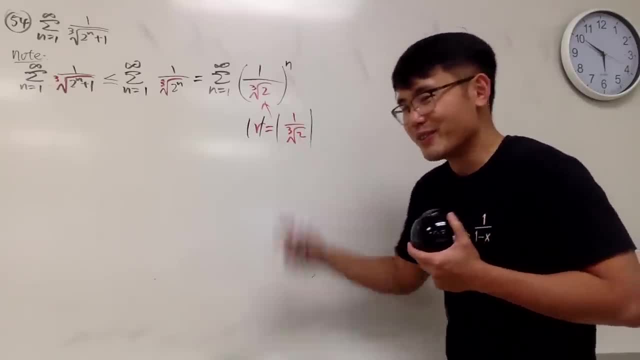 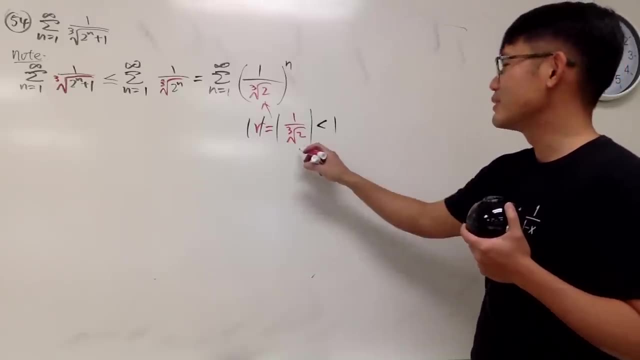 well, of course, 2 is bigger than 1.. The cube root of 2 is also bigger than 1.. So 1 over this is going to be less than 1.. That's useful, huh, Because this right here will tell us. 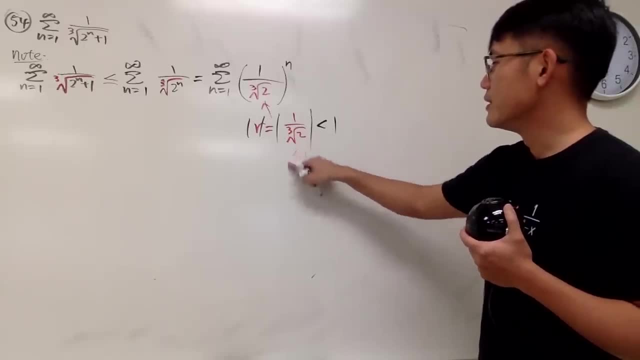 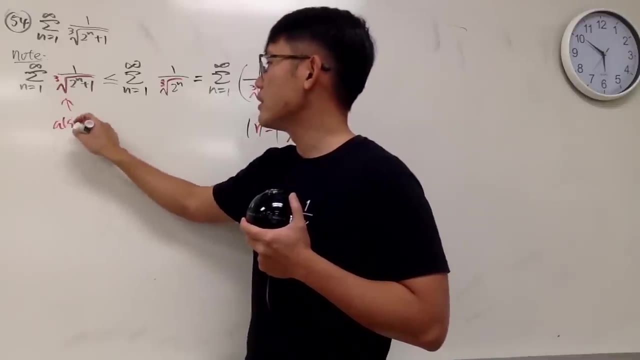 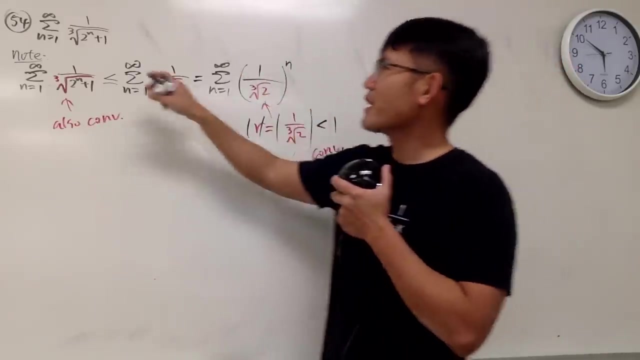 this right here is a converged situation. When I come back here, when I come back here, this right here also converges. And again when I put down r, I meant to say that your matrix series converges. So we can come back here and say: 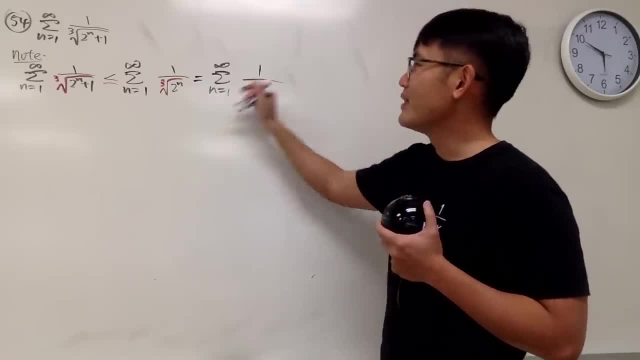 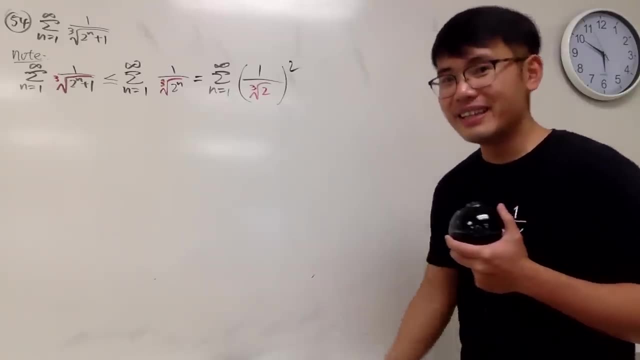 Cube root of 2, cube root of 2, like this. And then the nth power, And then we can just put the nth power on our side, like that. Very nice, huh. And now we are doing two things. 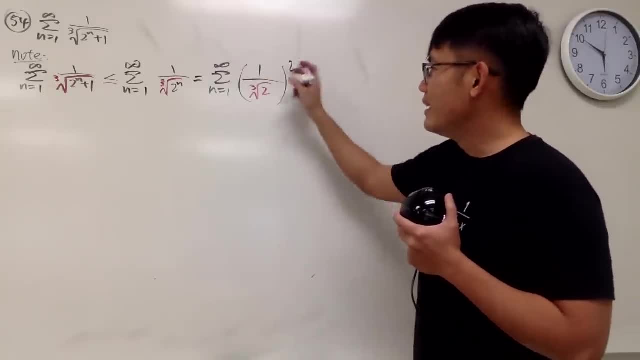 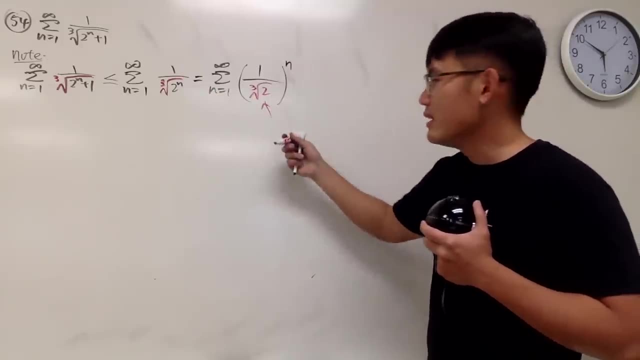 As you can see, this right here is what This right here is actually. oops, not a: 2, n. This right here is the common ratio r, which is 1 over the cube root of 2.. 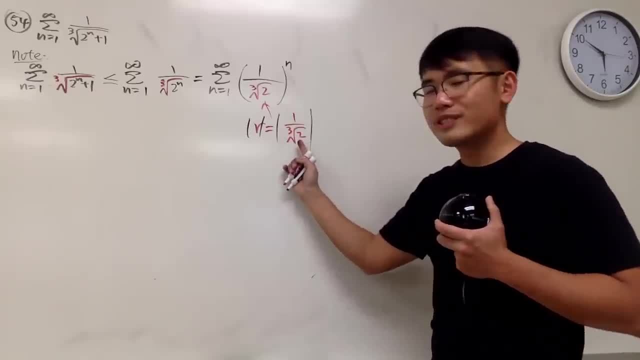 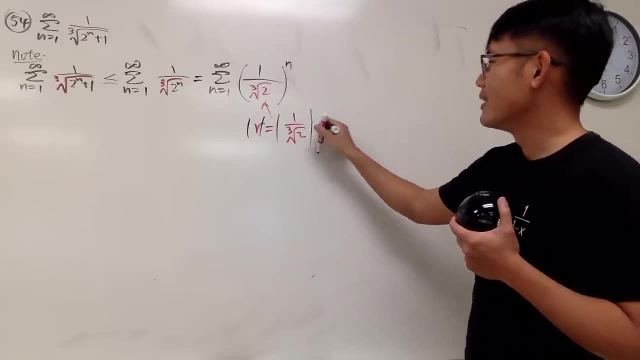 And if you take the absolute value, well, of course 2 is bigger than 1, the cube root of 2 is also bigger than 1.. So 1 over this is going to be less than 1.. That's useful. 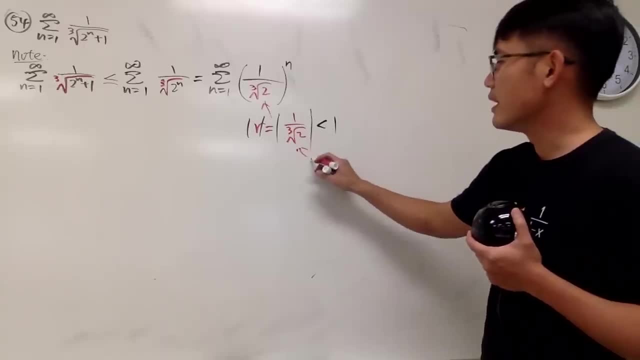 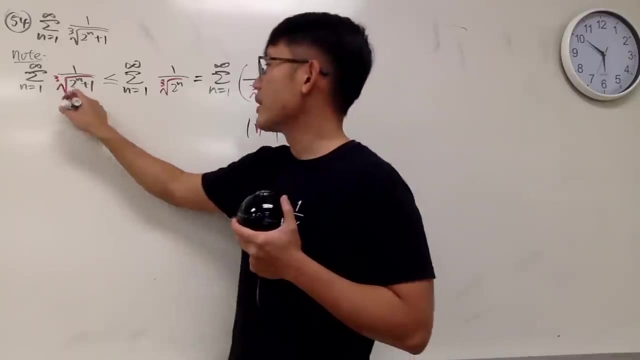 huh, Because this right here will tell us: this right here is a converged situation When I come back here. when I come back here, this right here also converges. And again, when I put on r, I meant to say the geometric series converges. 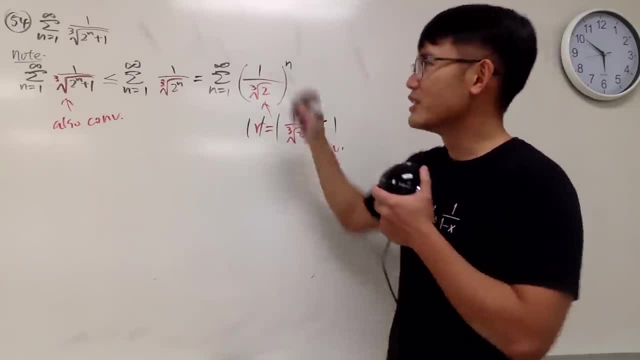 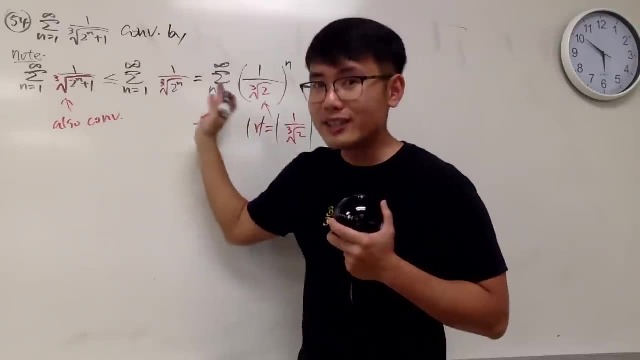 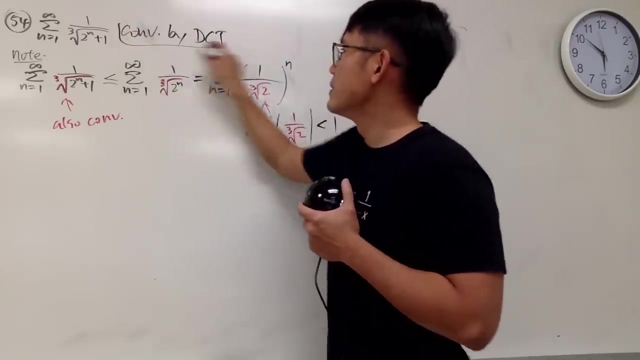 So we can come back here and say this: right, here is what Convergent, right Convergent by comparison with this guy. Comparison, because we're using inequality by direct comparison. test: Done, Done, done, done. 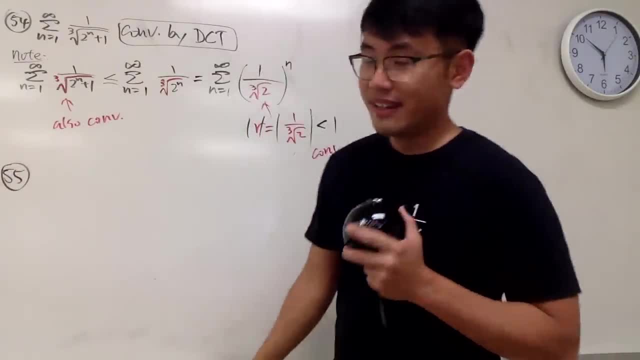 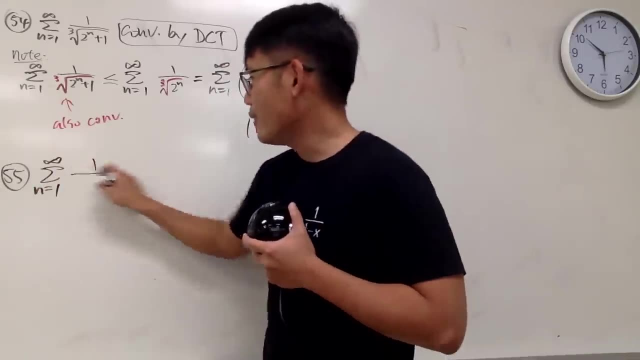 done Okay. number 55.. This right here, you guys will maybe hate it or maybe like it. up to you. Not integral, I almost wanted to say the integral 1 over the sum square root of n. natural log of n. 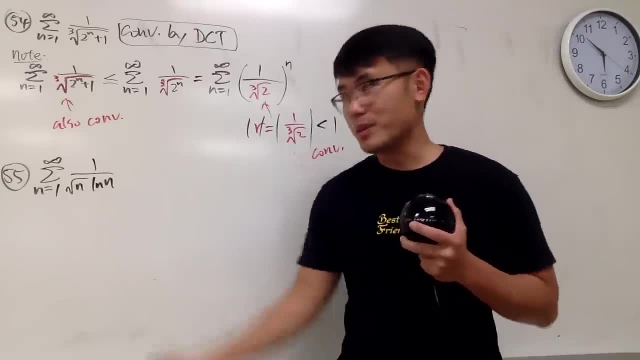 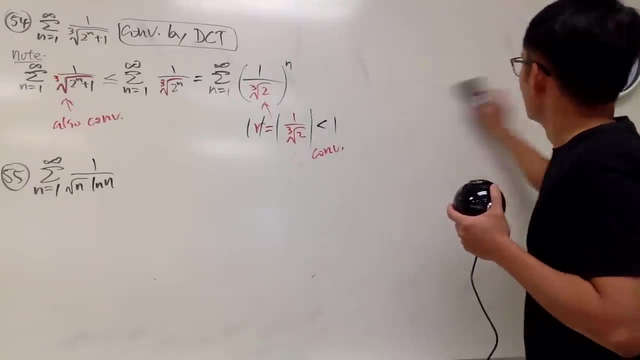 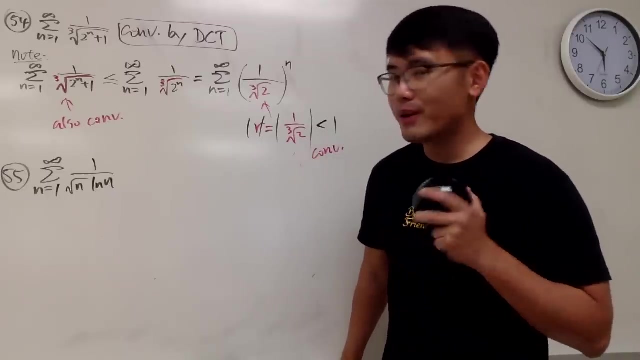 I know maybe you guys have seen this on your homework or maybe like your quiz, or maybe your test, but it's going to be on the final again. Think about it. I will erase the fourth. fourth right here. Okay. here's the DL: You cannot integrate 1 over square root of x, ln, x, And if you do direct comparison test with this, that still doesn't work right And limit comparison test doesn't work there If you do a limit comparison test. 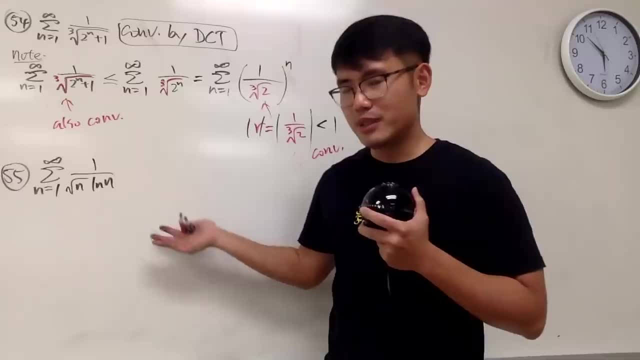 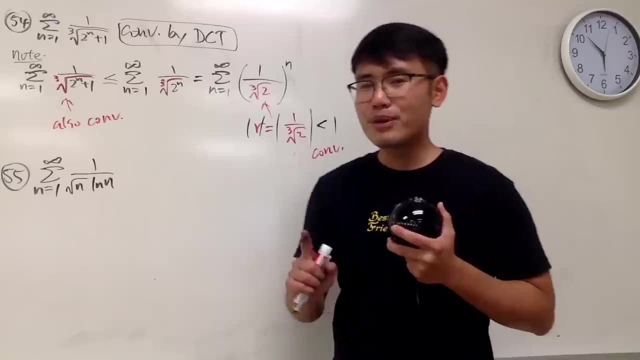 with 1 over square root of n, you end up with 0 or infinity, depends on how you put it, Not, not good? If you remember the list, let me tell you guys the following: This is like the secret, secret weapon. 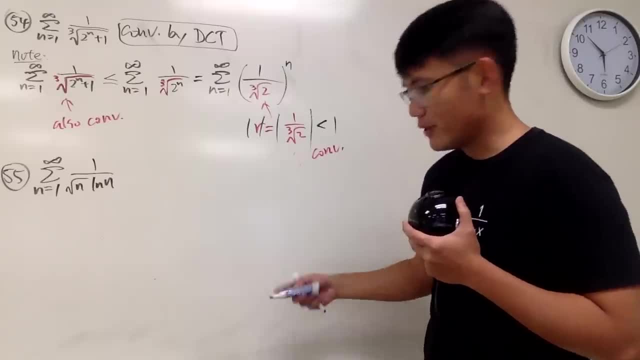 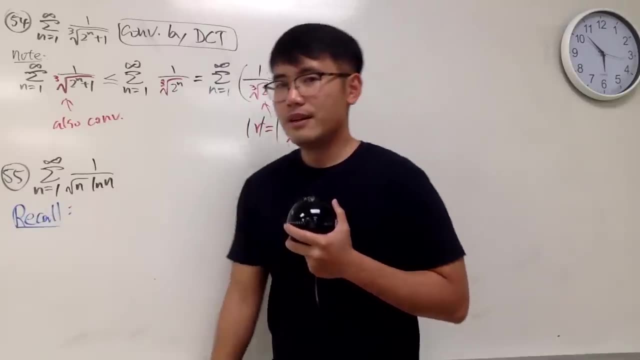 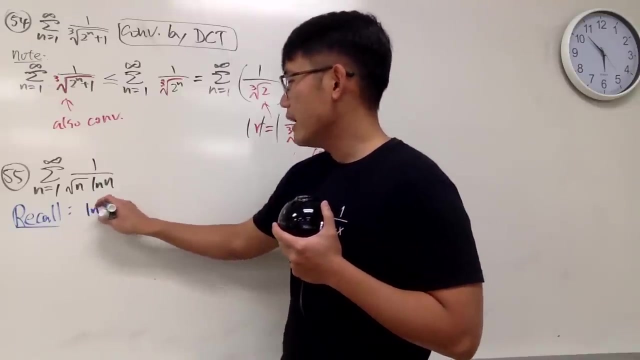 okay, So I will just put this down right here for you guys. Recall right From the list: we know that ln n is the smallest infinity And let me tell you: ln n is less than, is less than, less than. 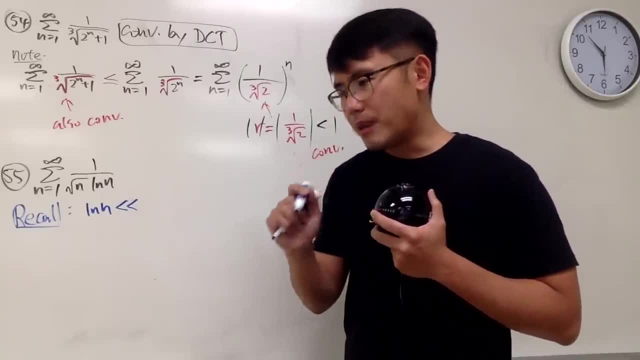 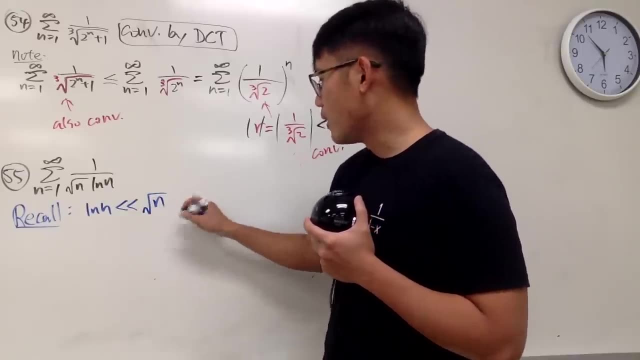 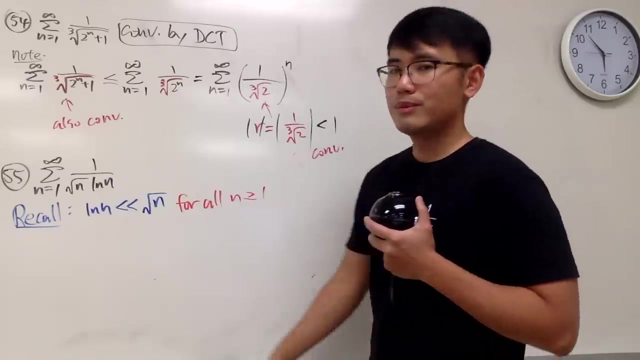 than x to some power And, in particular, I will tell you, is less than square root of n, And this is actually true for all n. Well, n is greater than or equal to 1, because n is a negative number, doesn't make sense. 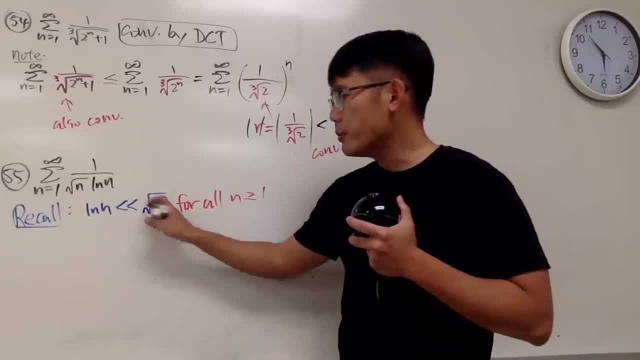 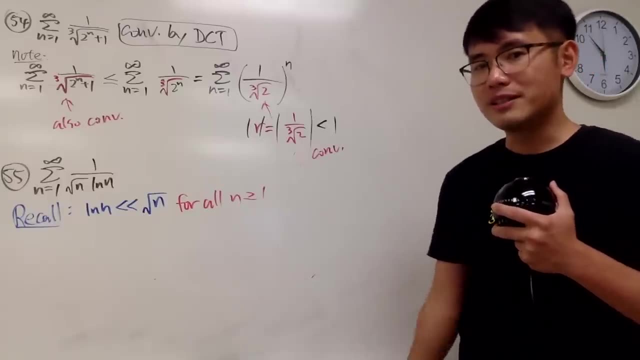 Okay, So this right here is actually always true. But if you use the cube root, okay, you have to actually pass some n value first, and then it will become true. But anyway, this is true. And now, how can we utilize this? 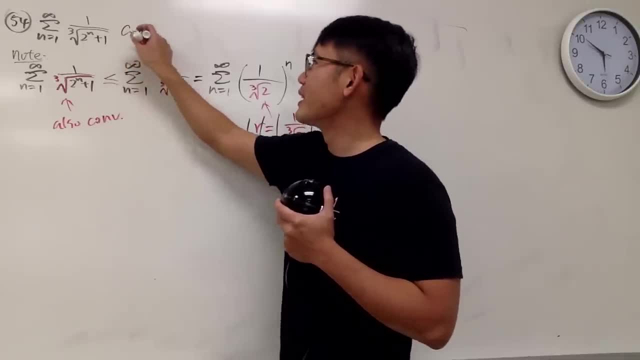 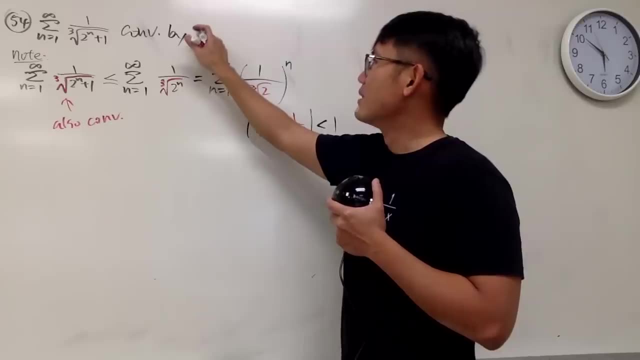 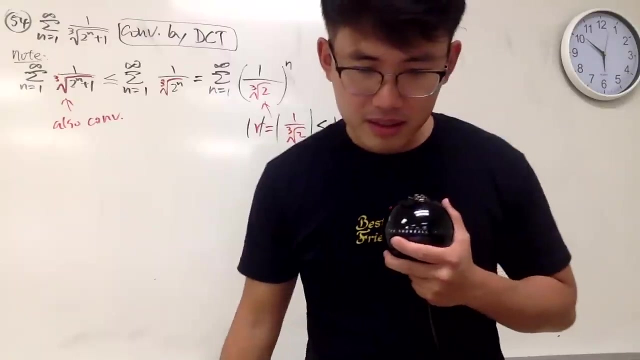 this right. here is what Convergent right. Convergent by comparison with this guy. Comparison because we're using inequality by direct comparison. test: Done, Done, done, done, done, done. Okay, number 55.. 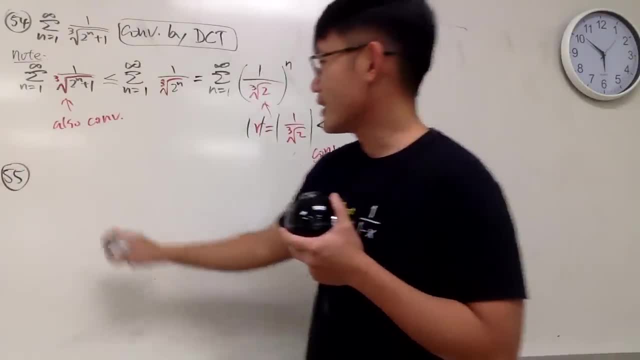 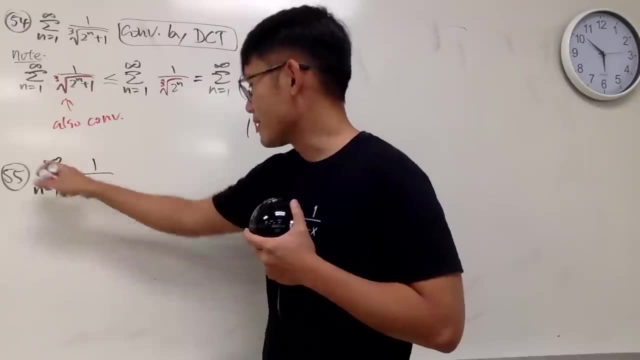 This right here. you guys will maybe hate it or maybe, like it's up to you, Not integral. I almost wanted to say integral 1 over the sum, okay, Square root of n. natural log of n. I know maybe you guys have seen this on your homework. 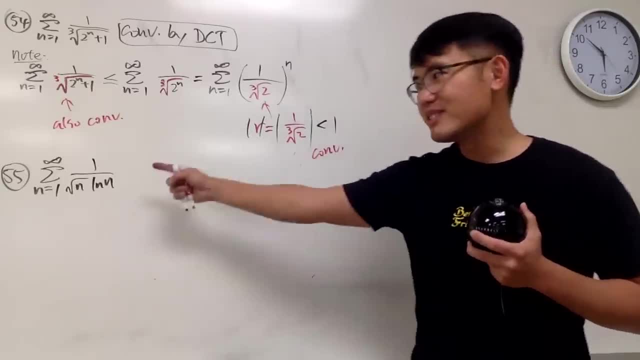 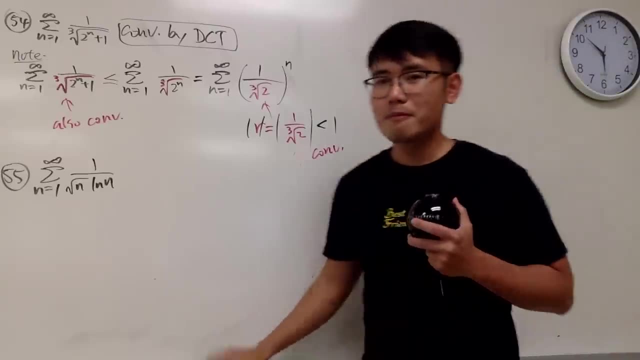 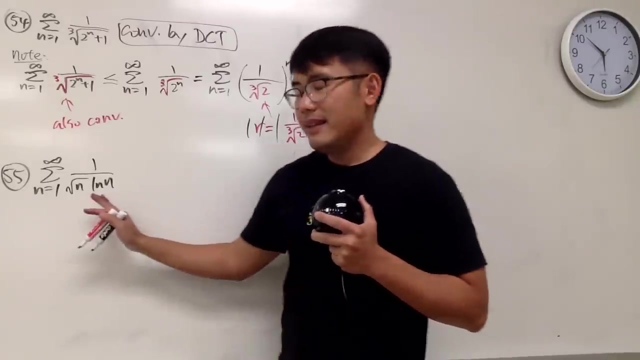 Or maybe like your quiz, or maybe your test, But it's going to be on the final again. Think about it. I will erase the fourth. Fourth, right here. Okay, here's the DL. You cannot integrate 1 over square root of x, ln, x. 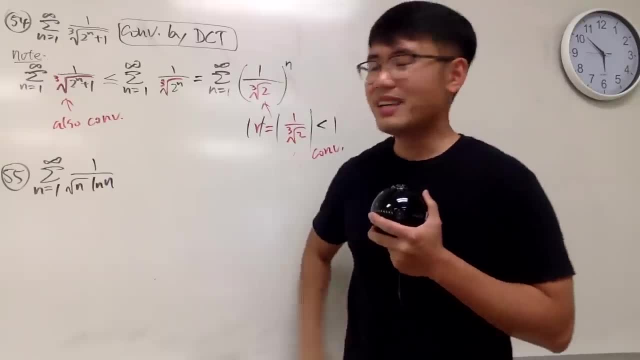 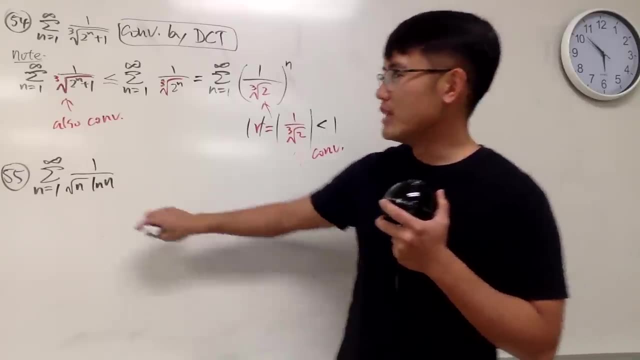 And if you do direct comparison test with this, what we'll start still doesn't work right, And limit comparison test doesn't work there. If you do a limit comparison test with 1 over square root of n, you end up with 0, or infinity, depends on how you put it. 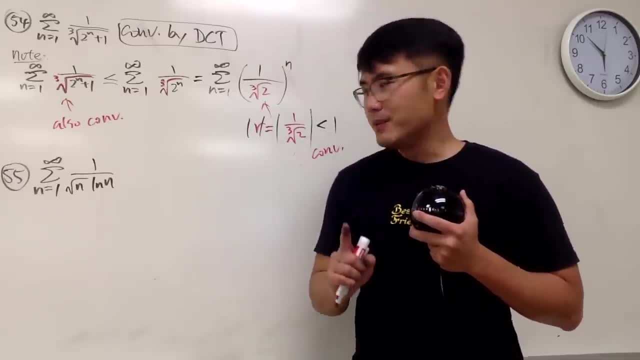 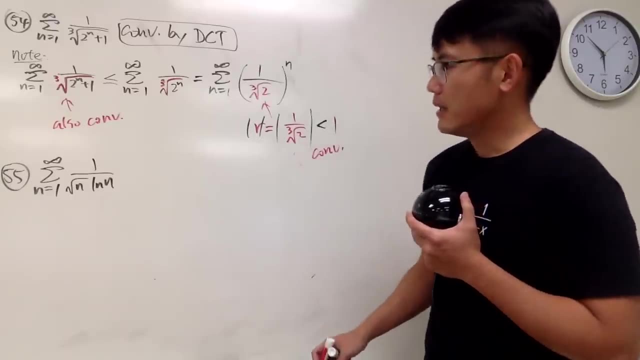 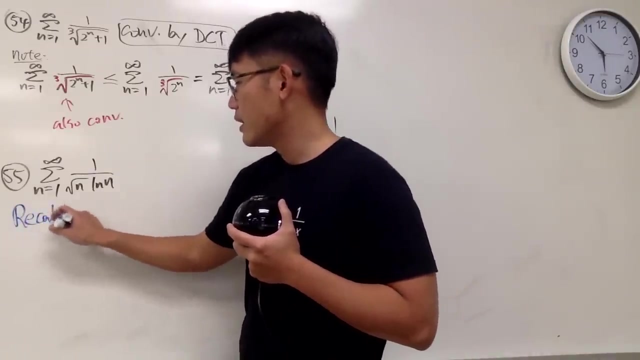 Not, not, not good. If you remember the list, let me tell you guys the following: This is like the secret secret weapon, okay, So I will just put this down right here for you guys. Recall right From the list: we know that ln n is the smallest infinity. 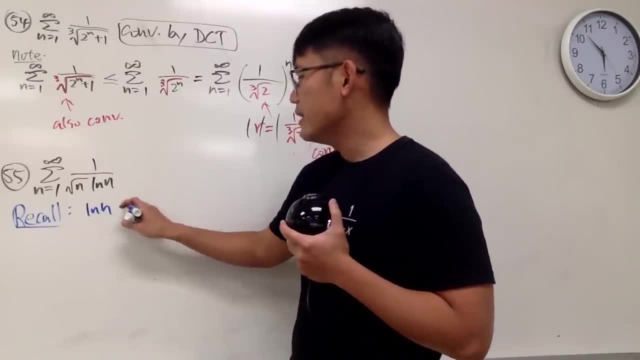 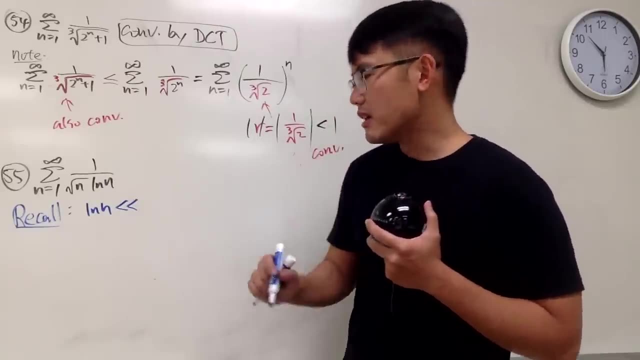 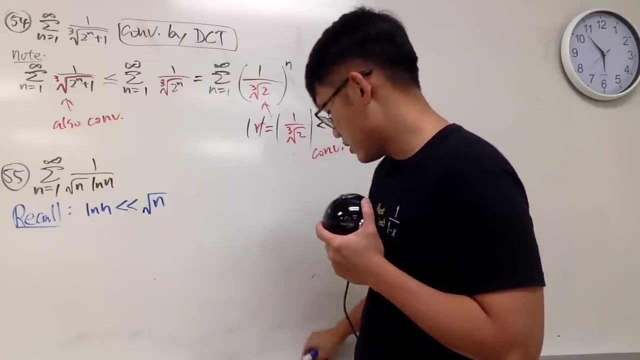 And let me tell you ln n is less than or less, is less than less than than x to some power And, in particular, I will tell you, is less than square root of n, And this is actually true for all n. 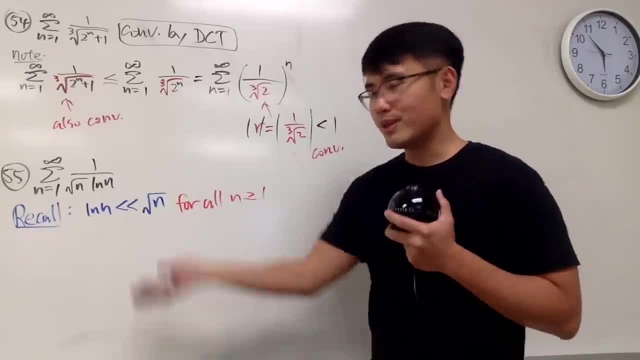 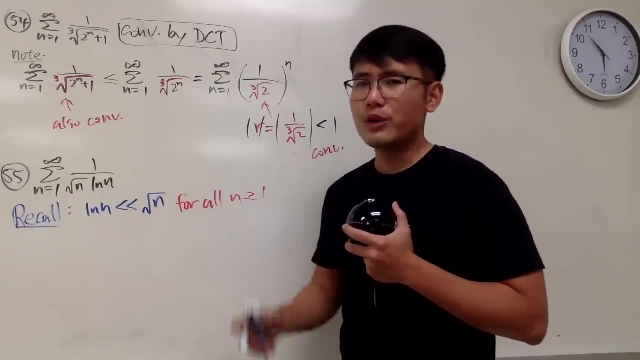 Well, n is greater than or equal to 1.. Because n is a negative number doesn't make sense. Okay, so this right here is actually always true. But if you use the cube root, okay, you have to actually pass some n value first. 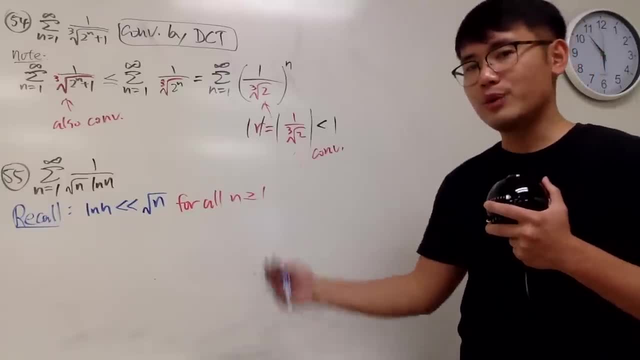 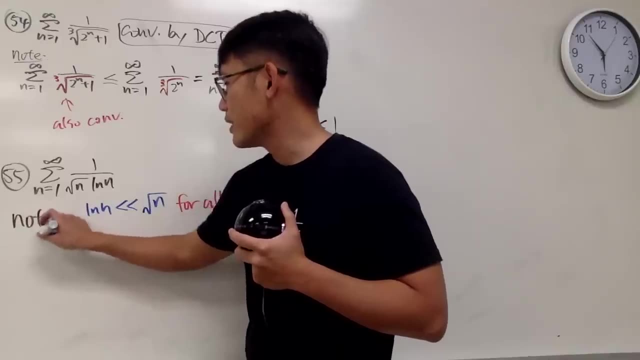 and then it will become true. But anyway, this is true. And now, how can we utilize this? Well, actually, I shouldn't say recall, I'll just say note, This sounds better. I'll just say note, Now, take the reciprocal on both sides. 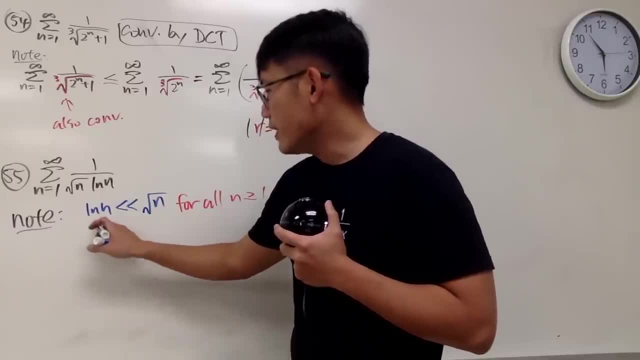 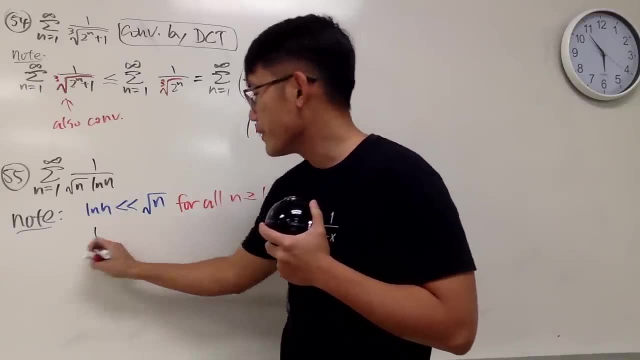 Check this out. I'll show you. If we take the reciprocal and both of them are positive, right, So we can just take the reciprocal and just flip the inequality symbol. 1 over ln n. 1 over ln n. 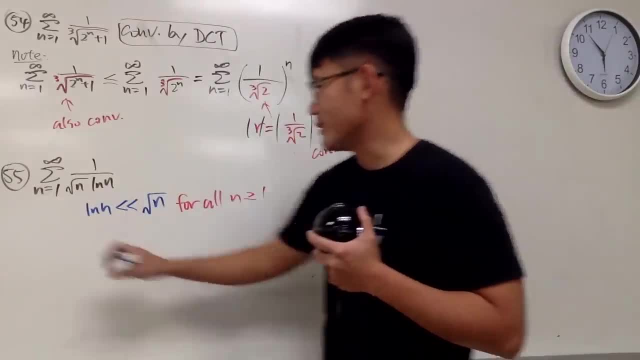 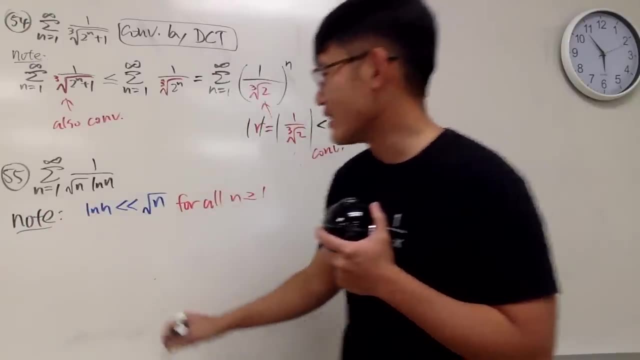 Well, actually I shouldn't say recall, I'll just say note. This sounds better. I'll just say note. Now take the reciprocal on both sides. Check this out, I'll show you If we take the reciprocal and both of them. 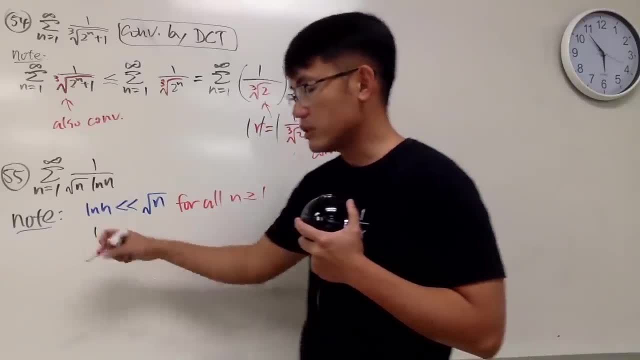 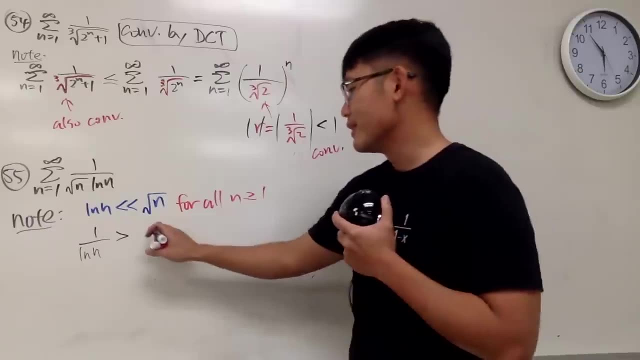 are positive, right, so we can just take the reciprocal and just flip the inequality symbol 1 over ln, n. And now I'm just going to write down: 1 greater than okay, it's none of this anymore Like this. 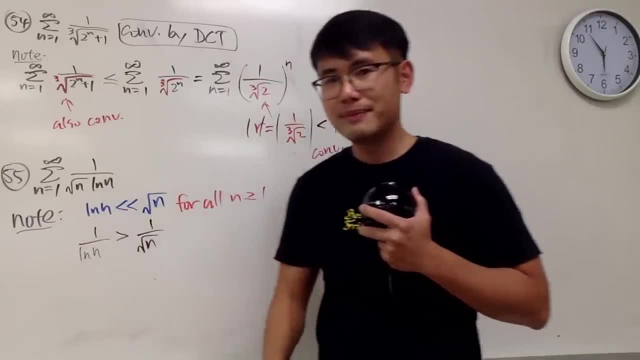 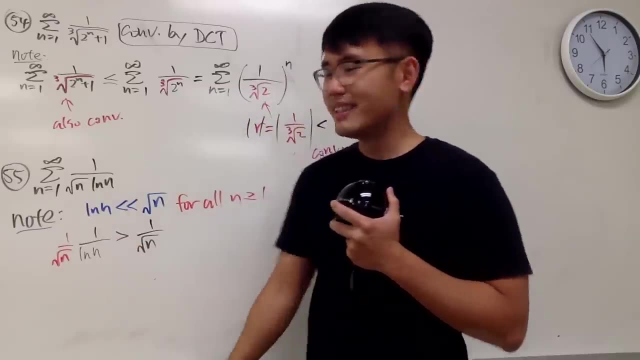 Ah, don't they look alike. Why don't we multiply both sides by 1 over square root of n, so that this is the same as that, And when we do that on the right-hand side, multiply by 1 over square root of n. 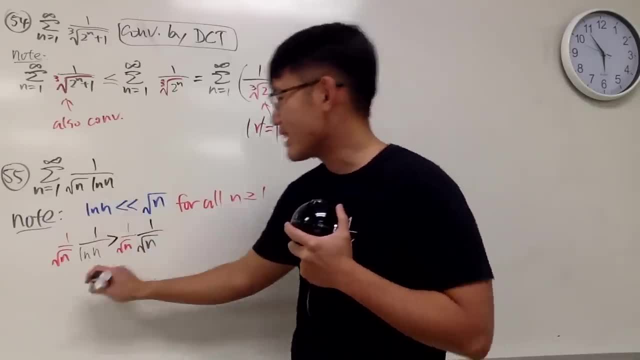 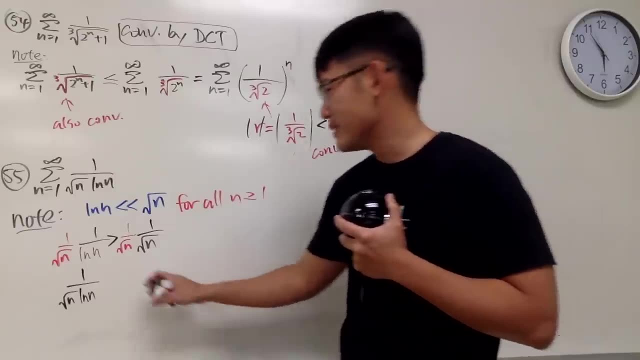 like this: What happens? The left-hand side is exactly what we want- 1 over square root of n, ln, n- And then the right-hand side is 1 over n And we just build up an inequality. This, right here, was a bad inequality. 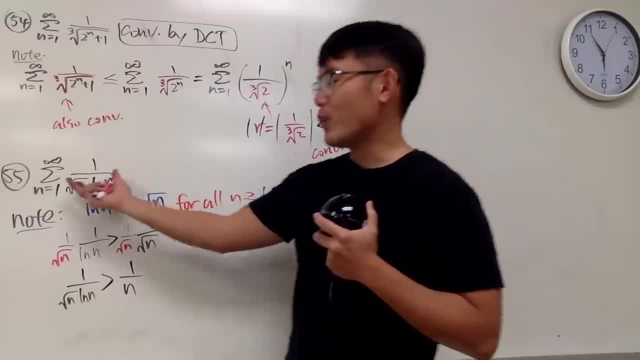 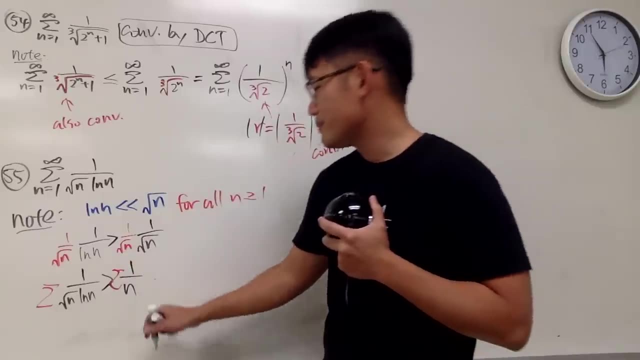 We just build up an inequality that the one that we want is bigger than the divergent that we know. So of course in the end we can just add our little summation here. Let me show you This right here is the harmonic series. 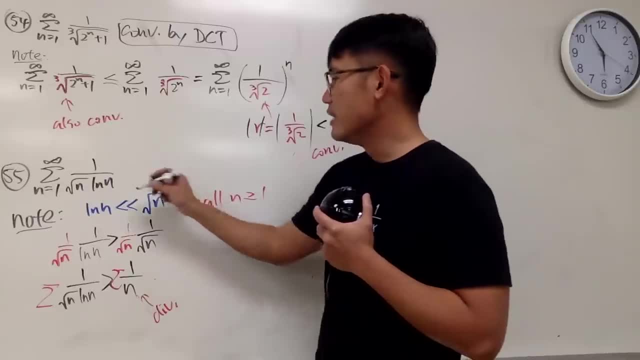 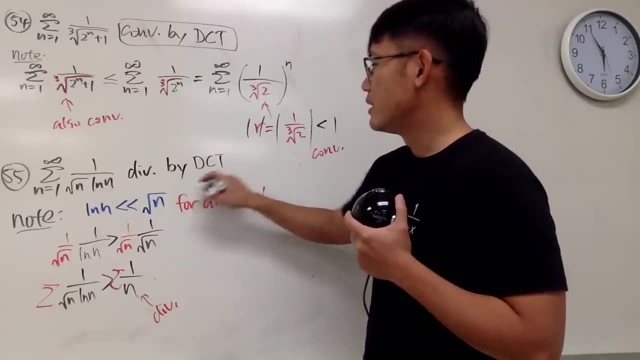 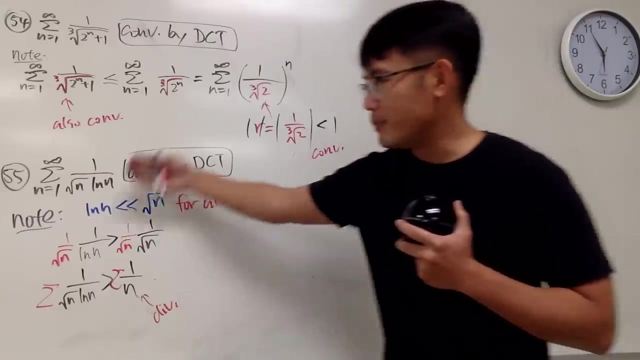 diverges of course, So we can come back here and say this: right here: diverges as well by direct comparison test, Right? So if you just use this and that it doesn't work, But with 1 over n it works out nicely. 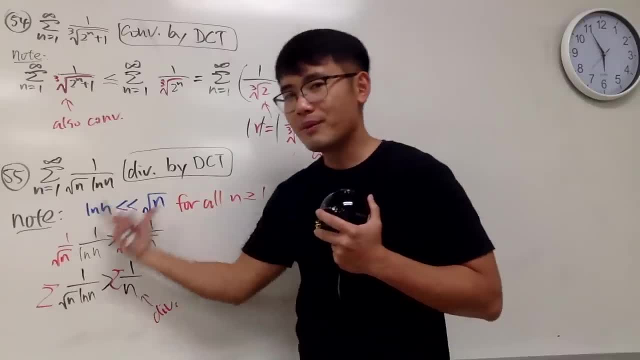 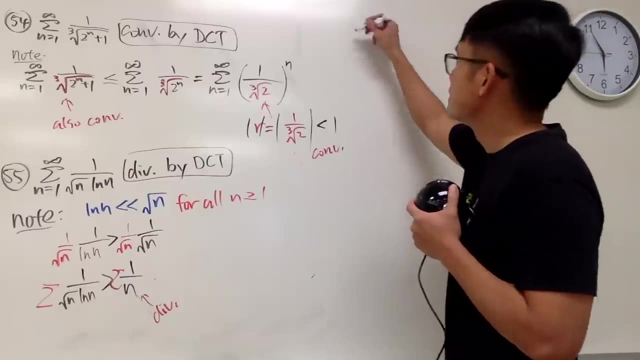 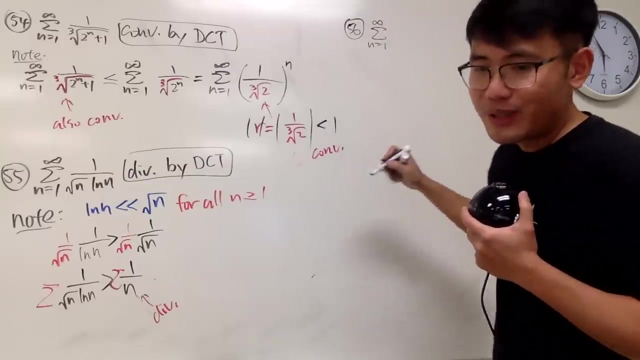 by building up steps like this. So this right here is a secret weapon. It's pretty useful. OK, Now let's see Number 56. So we are going to do the sum as n goes from 1 to infinity, And we have. 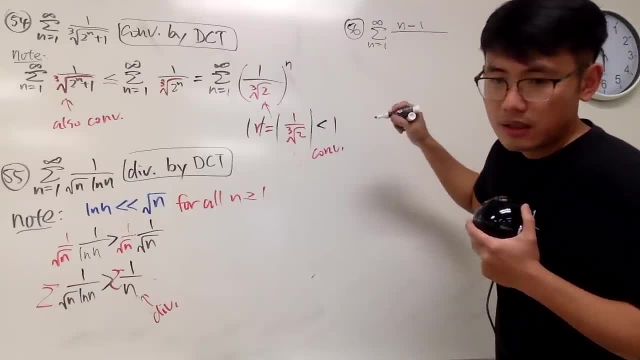 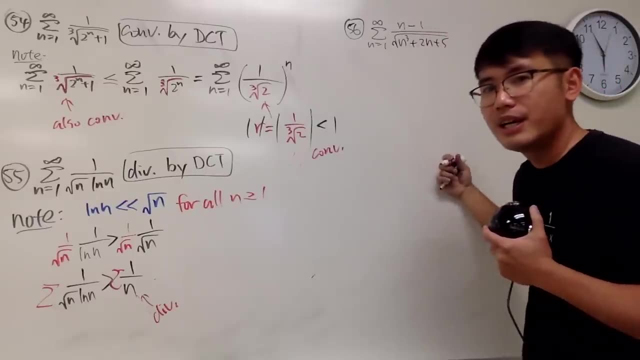 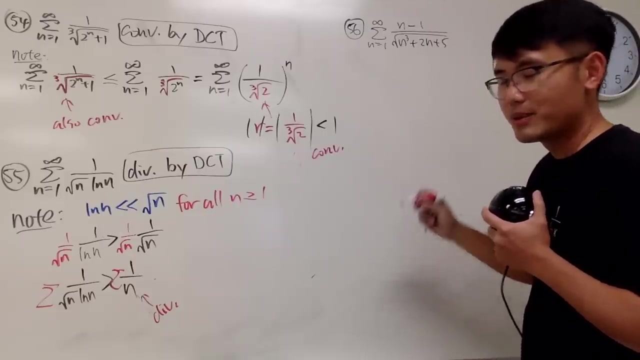 n minus 1 over the n, the square root of n, cubed plus 2n plus 5, like this: Well, I think for this one, I'm just going to let you guys try. OK, I'm going to let you guys. 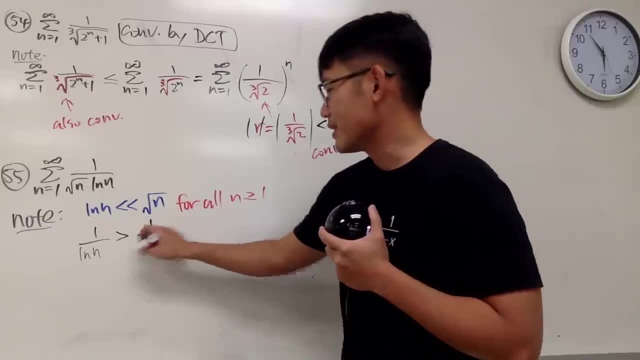 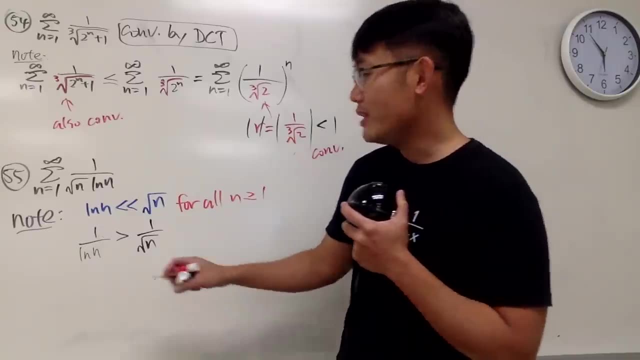 And now I'm just going to write down 1 greater than It's. none of this anymore Like this: Ah, don't they look alike? Why don't we multiply both sides by 1 over square root of n, so that this is the same as that? 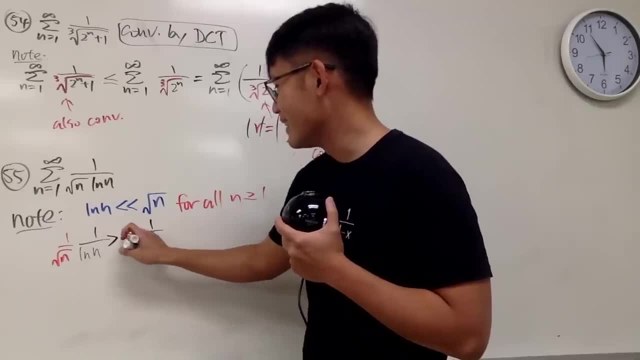 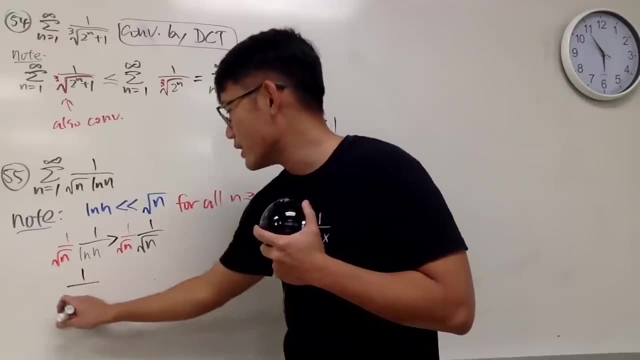 And when we do that on the right-hand side, multiply by 1 over square root of n, like this: What happens? The left-hand side is exactly what we want: 1 over square root of n. 1 over square root of n. 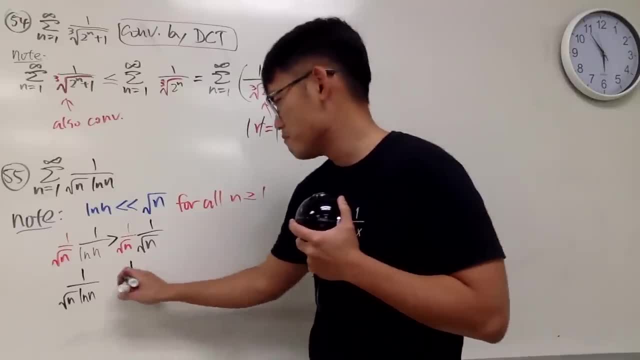 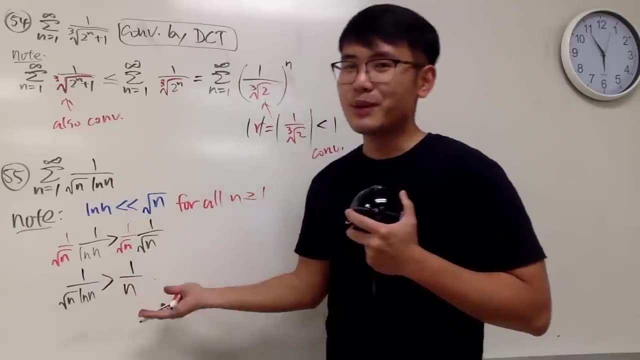 And then the right-hand side is 1 over n And we just build out an inequality. This, right here, was a bad inequality. We just build out an inequality that the one that we want is bigger than the divergent one we know. So, of course, in the end, 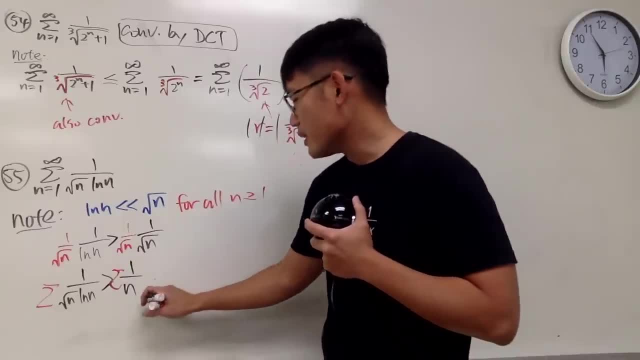 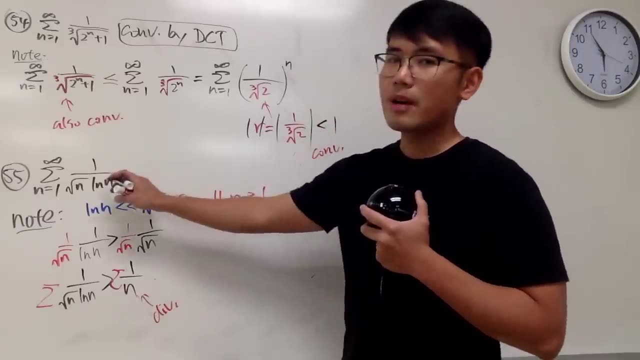 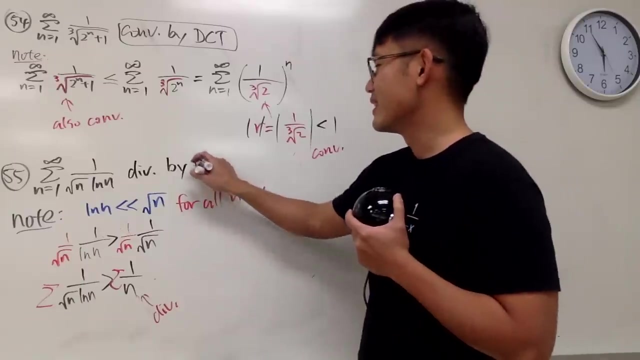 we can just add our little summation here. So I will just tell you this: right here is the harmonic series Diverges, of course. So we can come back here and say this: right here diverges as well by direct comparison test. 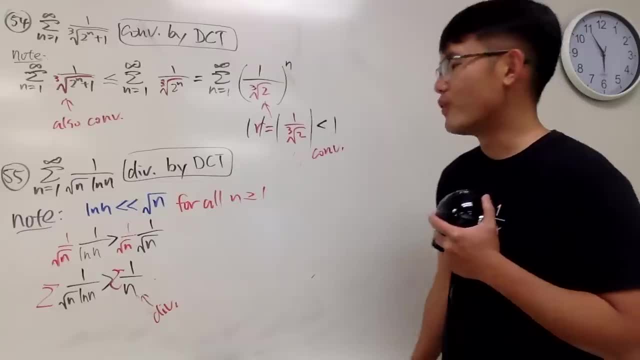 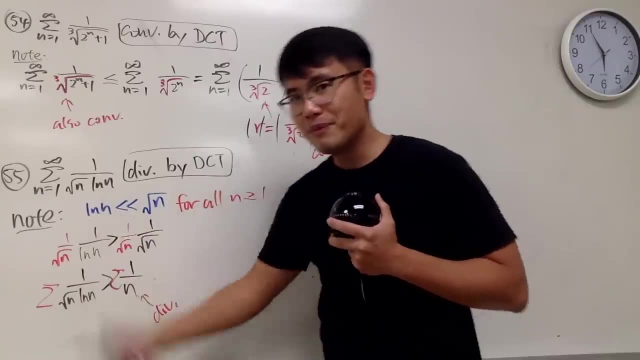 Right. So if you just use this and that, it doesn't work, But with 1 over n, it works out nicely by building up steps like this. So this right here is a secret weapon. It's pretty useful, Okay. 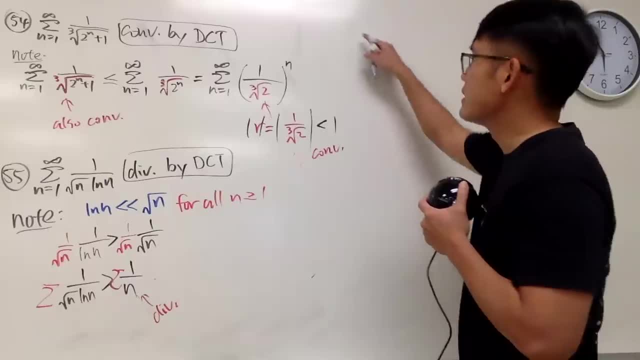 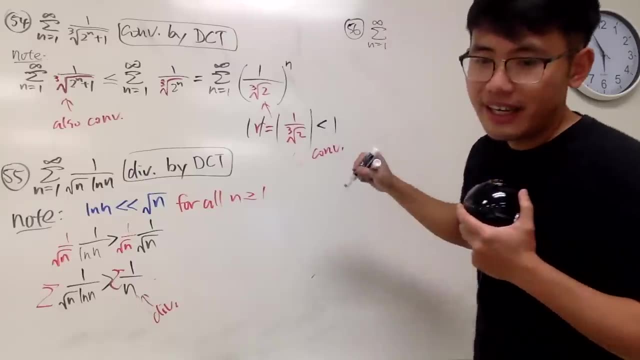 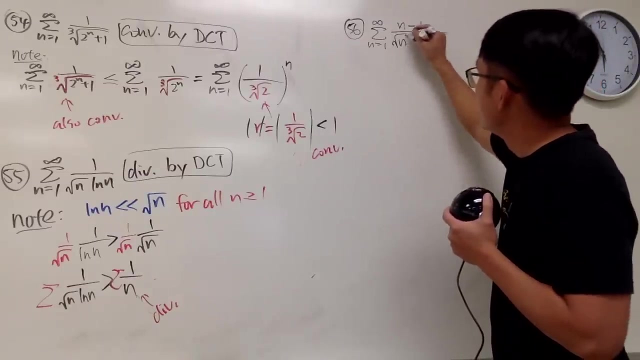 Now let's see Number 56.. So we are going to do the sum as n goes from 1 to infinity and we have n minus 1 over the square root of n, cubed plus 2n plus 5, like this: 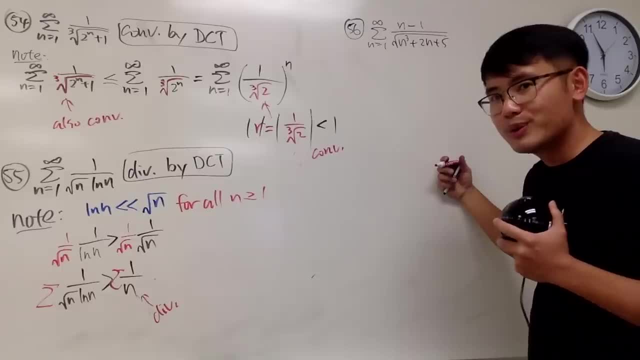 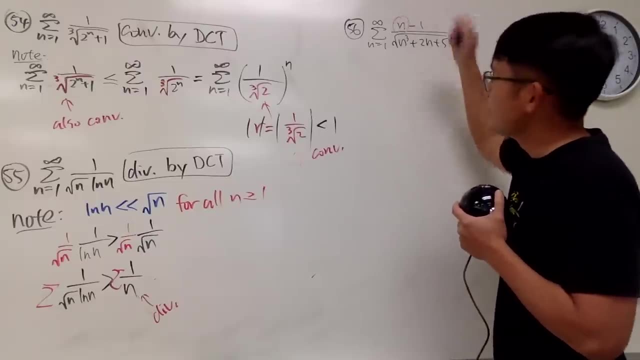 Well, I think for this one I'm just going to let you guys try. Okay, for 56, I'm going to let you guys try to work out all the steps on your own. You see that here we can just look at the dominating part. 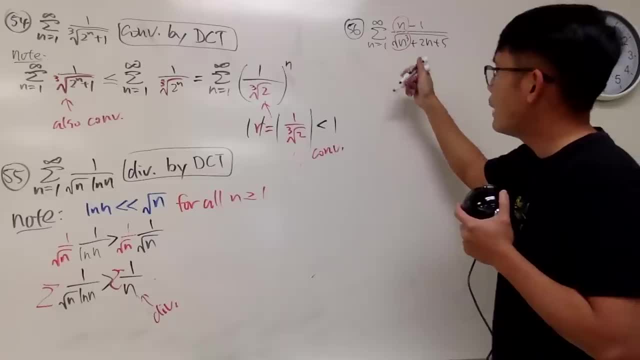 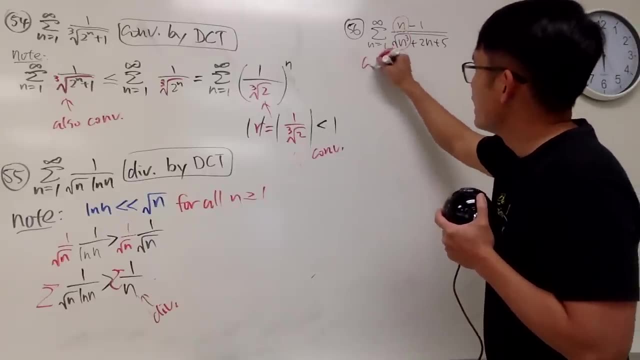 and here we can look at the dominating part right. So I will just give you guys a hint. You have to practice how to do this kind of things on the test, on your own right. Well, I will just tell you guys. 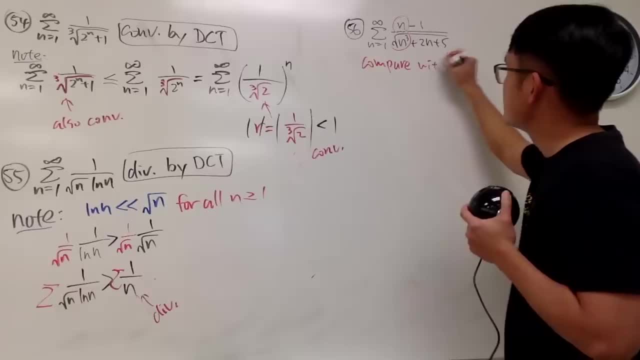 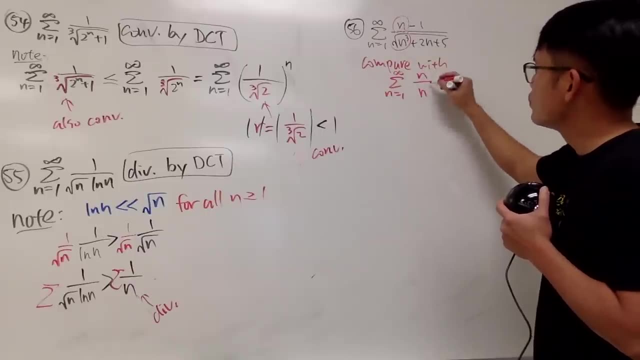 compare this with the sum as n goes from 1 to infinity, which is n over n, to the 3 over 2 power, like that, And of course this is the same as saying 1, which is 2 over 2,. 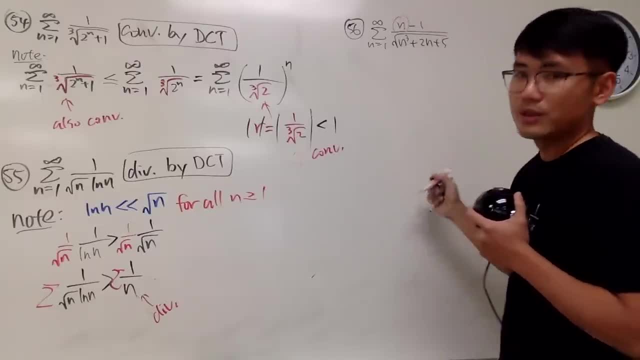 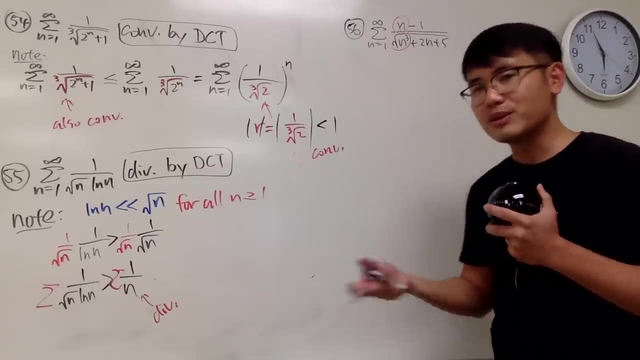 try to work out all the steps on your own. You see that here we can just look at the dominating part, And here we can look at the dominating part Right. So I will just give you guys a hint. You have to practice how to do this kind of. 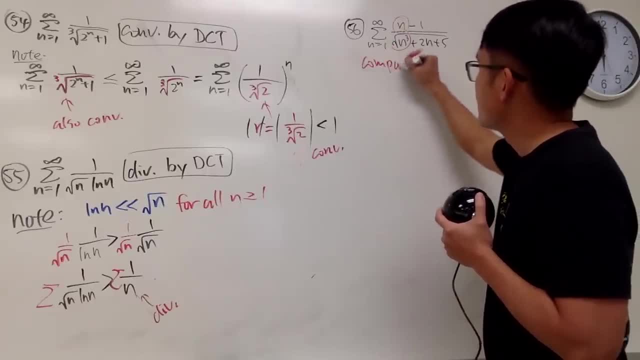 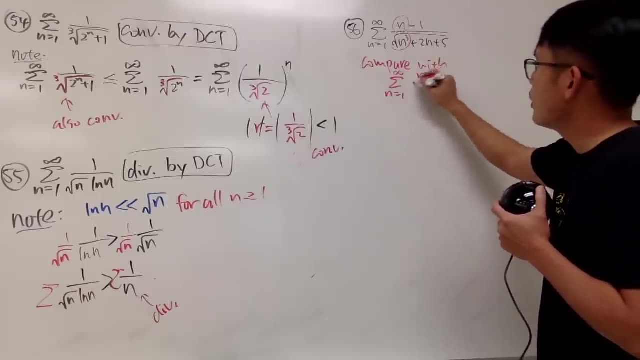 things on the test on your own Right. Well, I will just tell you guys, compare this with the sum as n goes from 1 to infinity, which is n over n, to the 3 over 2 power, And, of course, 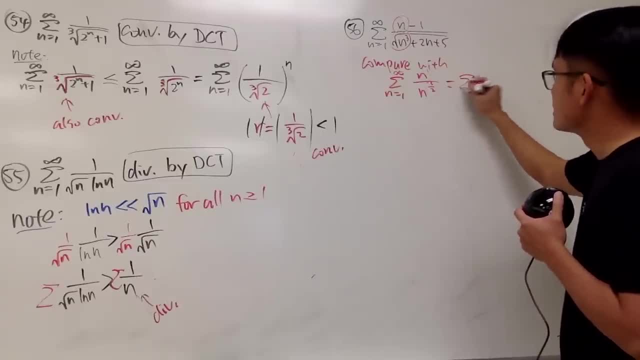 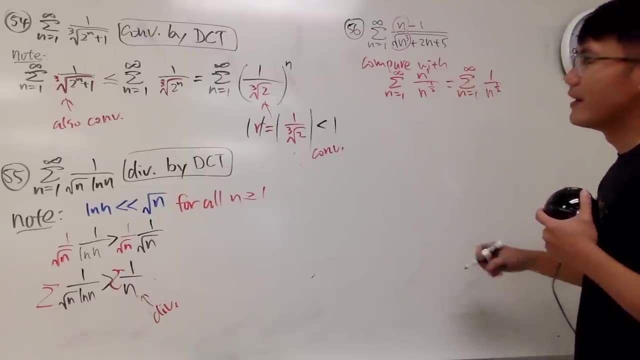 this is the same as saying 1,, which is 2 over 2,, which is the same as saying n goes from 1 to infinity and you have 1 over n to the 1 half power, Right, And in the end you will see that. 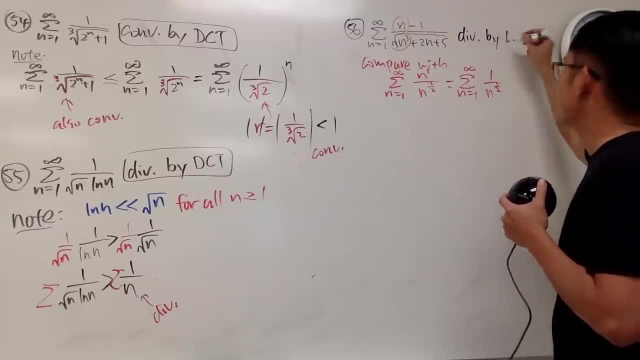 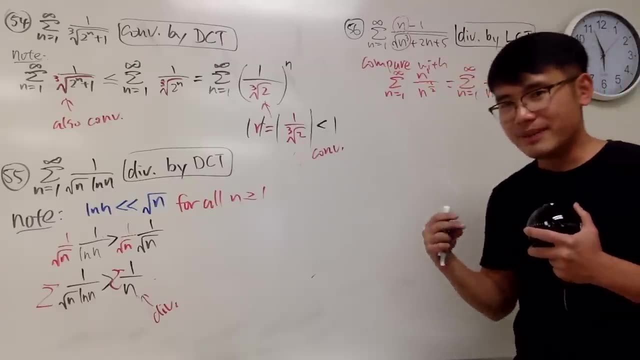 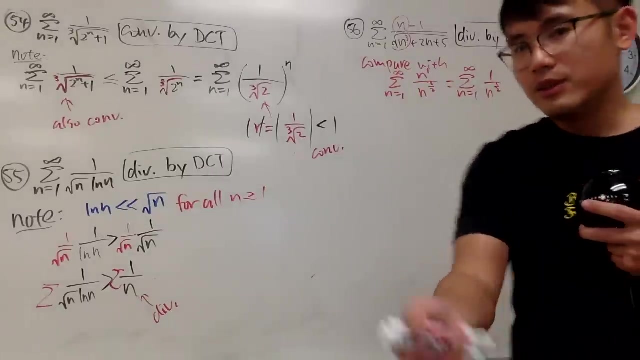 this right here diverges by limit. well, you can do limit comparison test or even direct comparison test. maybe works as well, but I will just say limit comparison test, right? So that would be the idea. You can just do that and then you show. 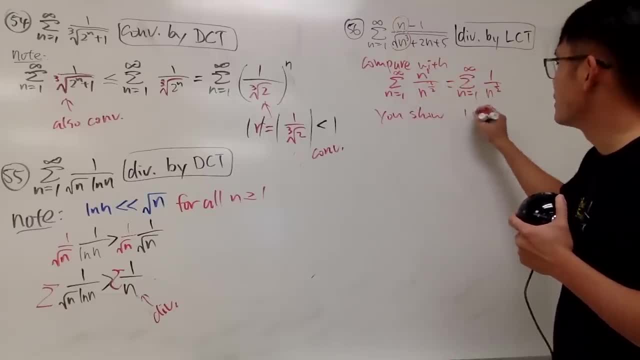 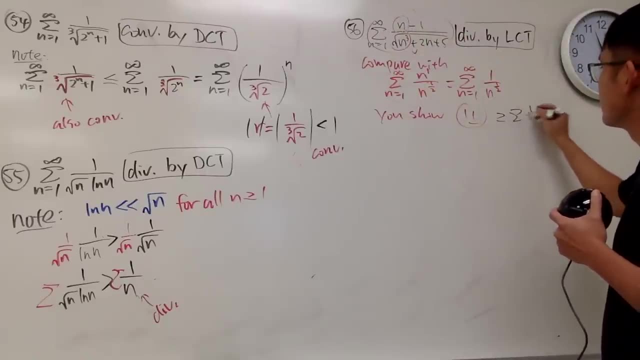 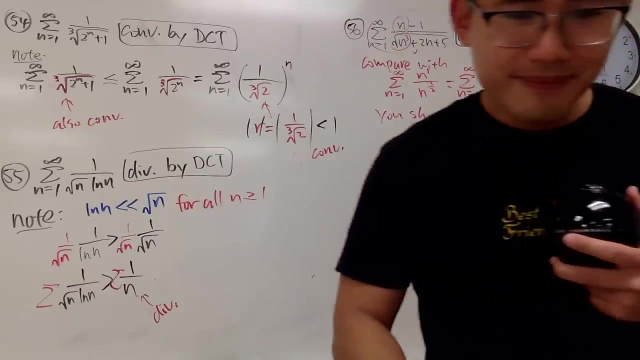 okay, you show this right here. the happy face right here. right, The happy face right here is bigger than or equal to the series as 1 over n squared, no, 1 over right, You show it Seriously. Another page done. 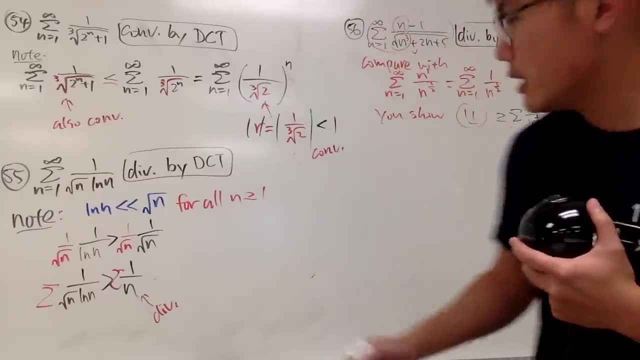 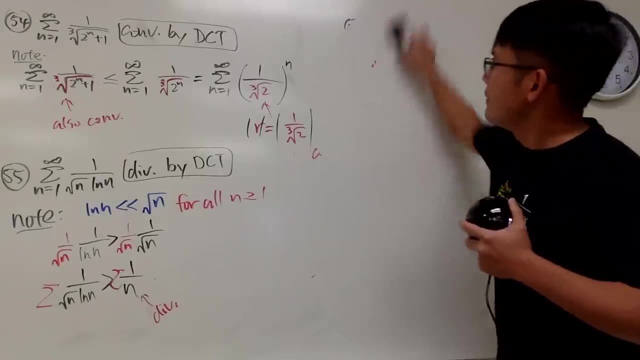 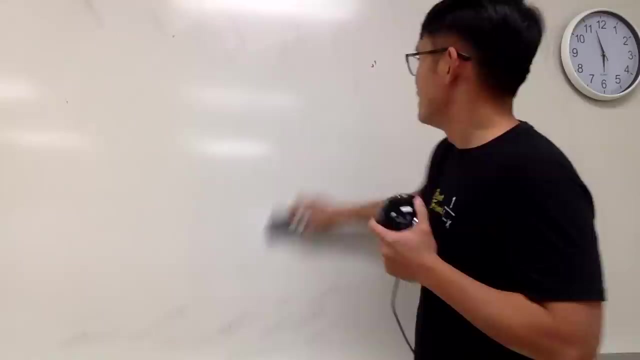 Two and a half more page to go Right. So we'll see how this goes And I am going to erase this Right. So seriously, the more you do this, the quicker you can get, and I don't have to, you know. 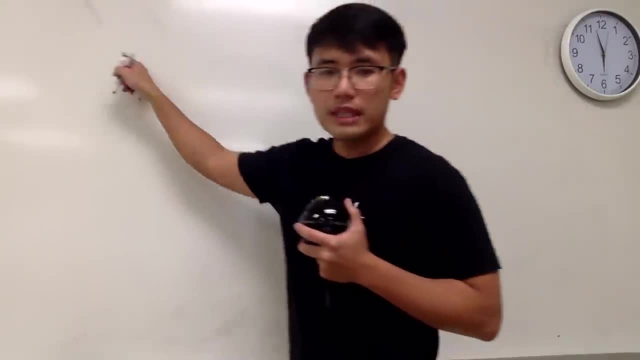 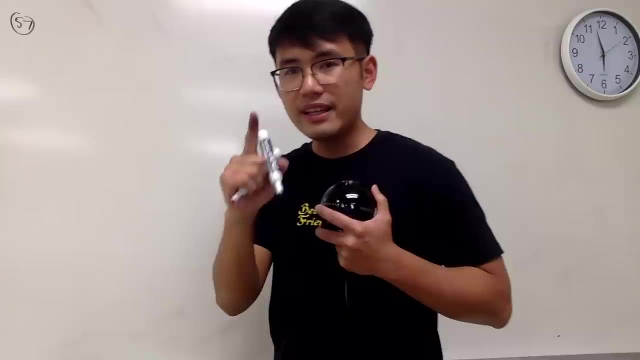 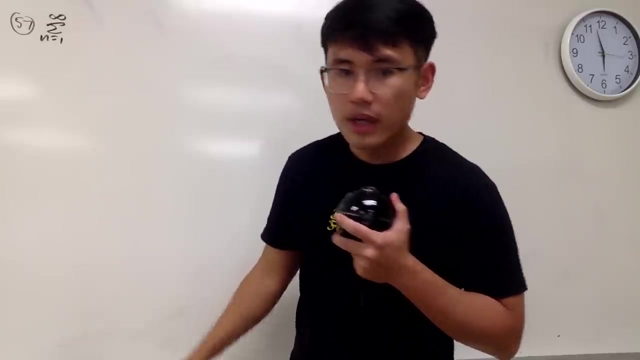 give you guys that much explanation, because a lot of things is really similar, Right? Let me know if you guys like integrals more or series more. Anyway, the sum as n goes from 1 to infinity, n squared times n times 2 to the. 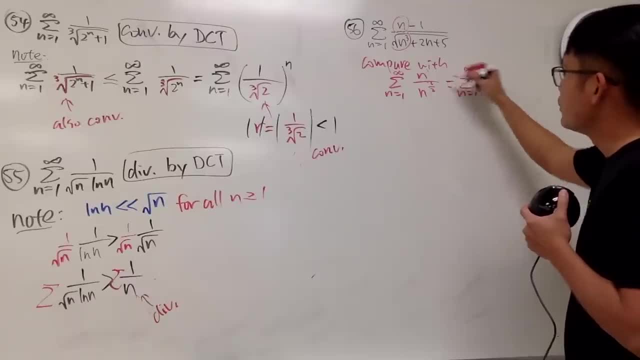 which is the same as saying n goes from 1 to infinity and you have 1 over n to the 1 over 2 power right. And in the end you will see that this right here diverges by limit. well, you can do limit comparison test. 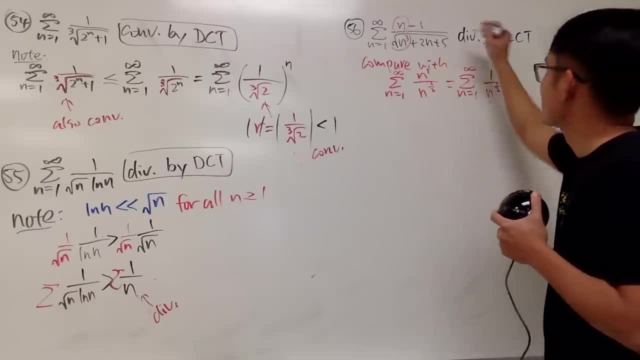 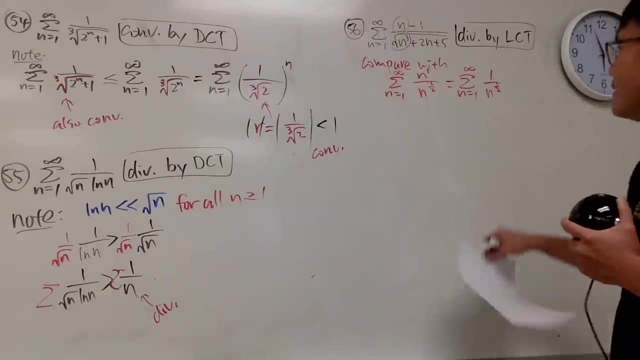 or even direct comparison test. maybe it works as well. but I will just say: limit comparison test because it's quicker that way, right? So that would be the idea. You can just do that and then you show, okay. 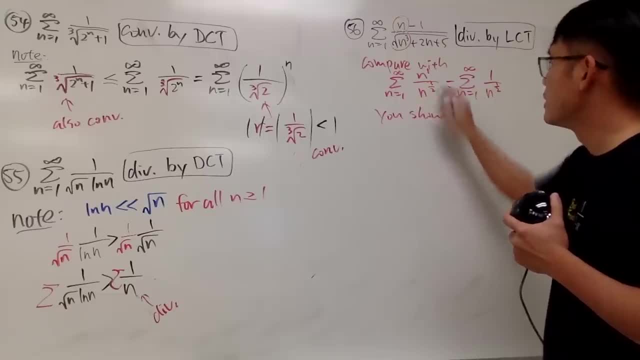 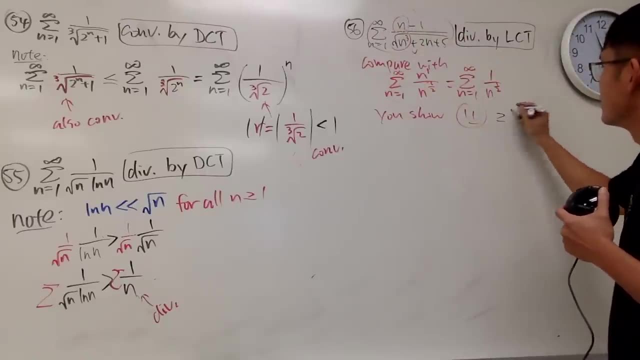 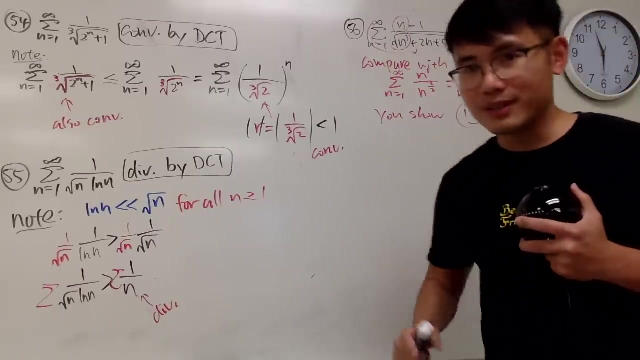 You show this right here. the happy face right here. the happy face right here is bigger than or equal to the series as 1 over n squared, no, 1 over right. You show it seriously. Another page done. 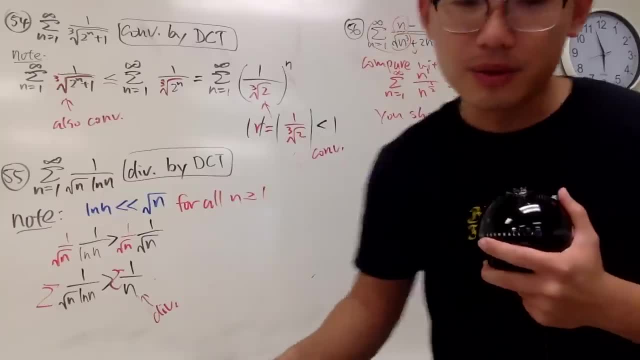 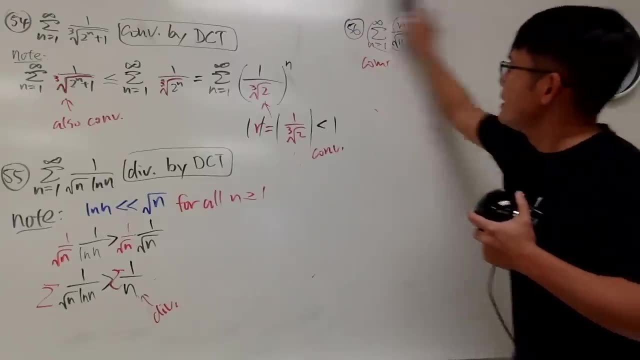 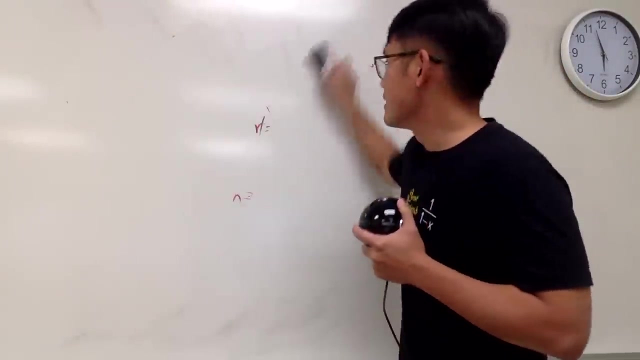 Two and a half more pages to go right. So we'll see how this goes And I am going to erase this right. So seriously, the more you do this, the quicker you can get, and I don't have to, you know. 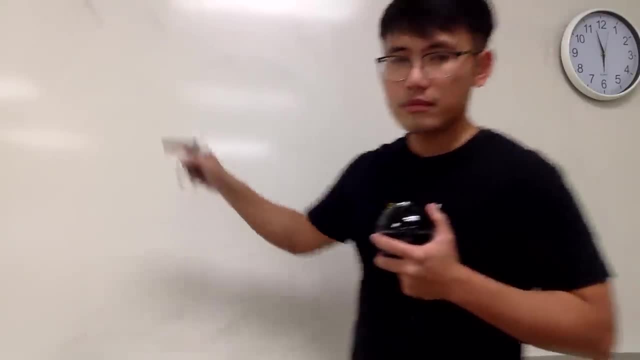 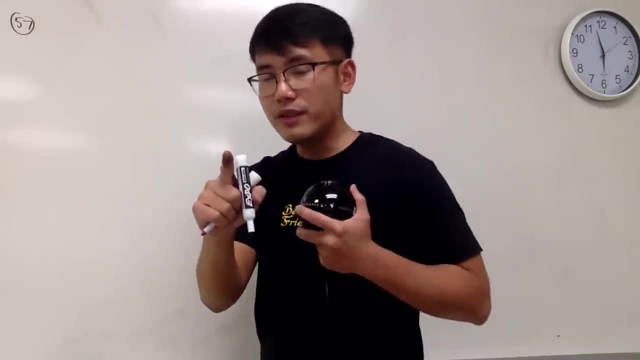 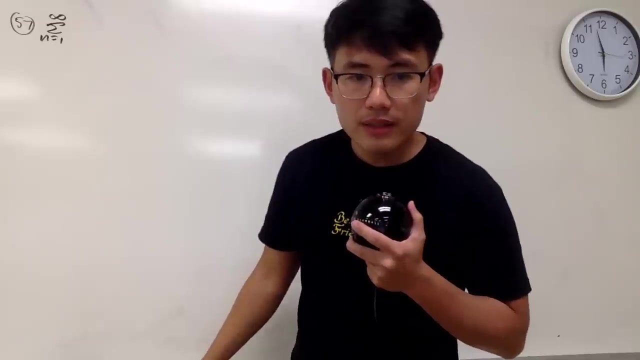 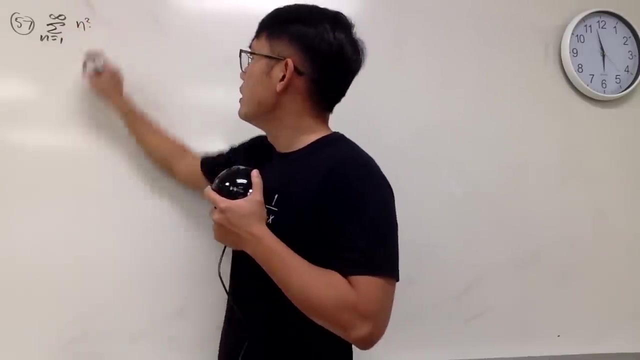 give you guys that much explanation, because a lot of things is really similar, right? Let me know if you guys like integrals more or series more. Anyway, the sum as n goes from 1 to infinity n squared times n times 2 to the n plus 2,. 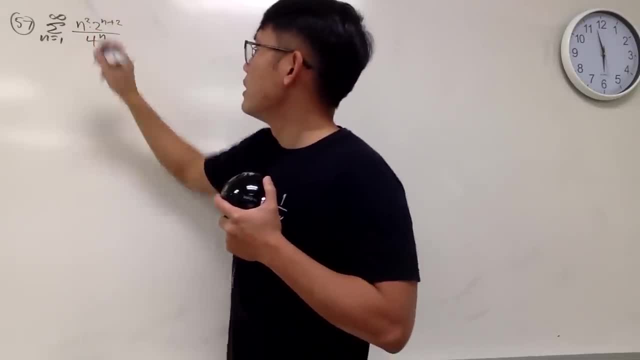 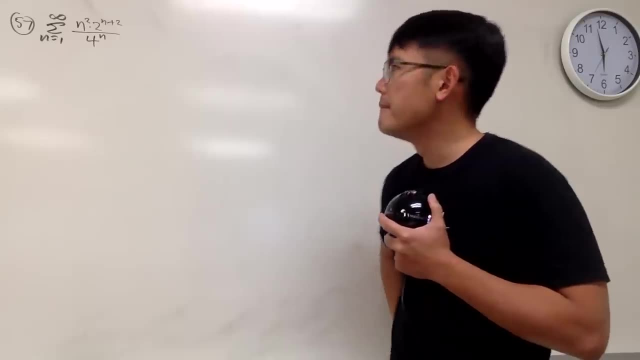 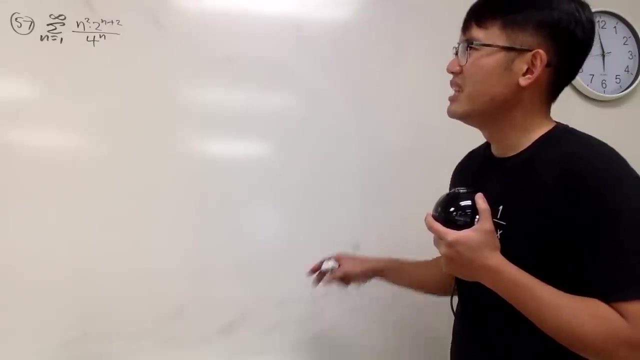 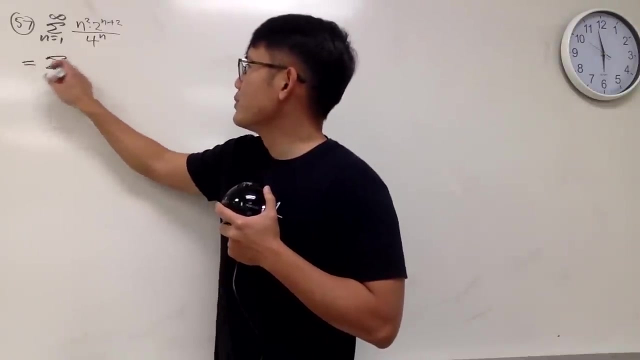 over 4 to the nth power, like that. Huh, God, Hmm, Let me just simplify the expression a little bit to make me feel better. okay, To make us feel better. So notice that. this right here. let's do some algebra right here. 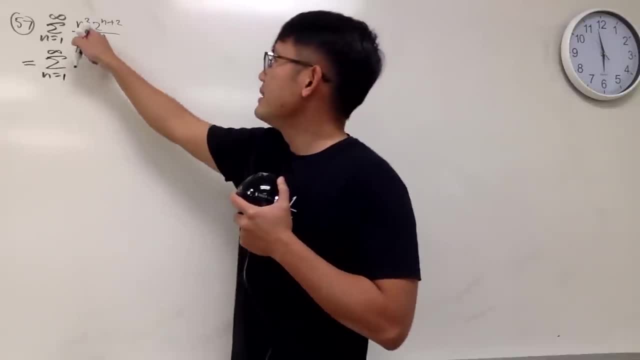 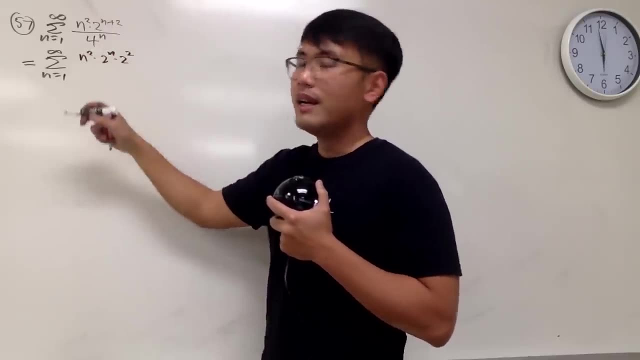 This is n equals 1 to infinity, and this is just n squared times. this is 2 to the n, and of course we can just say that's multiplied by 2 to the 2nd power, and on the bottom, if you would like, 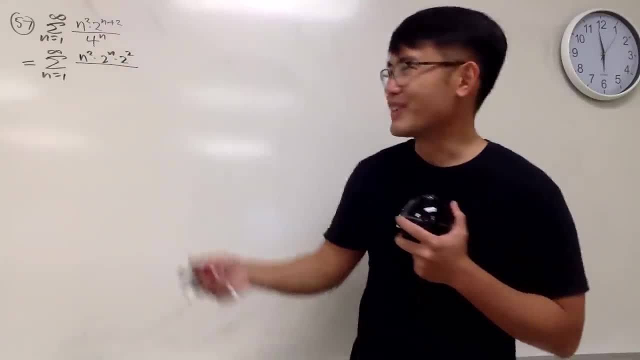 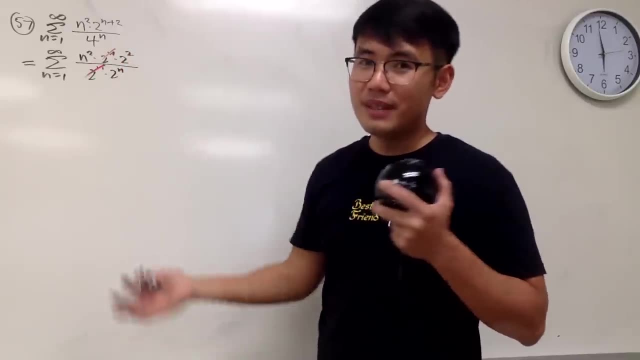 4 is the same as 2 times 2, so we can look at this as 2 to the n times 2 to the n, and the point is that I want to get rid of these two things. That's much better. 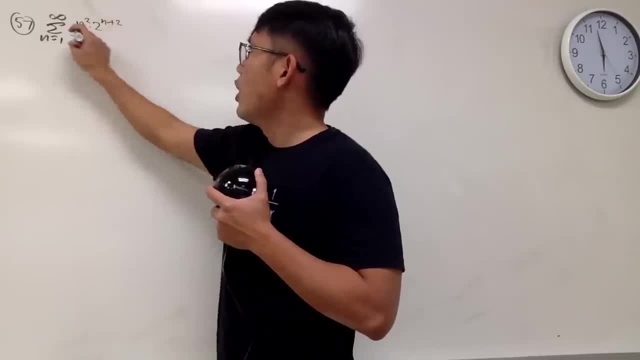 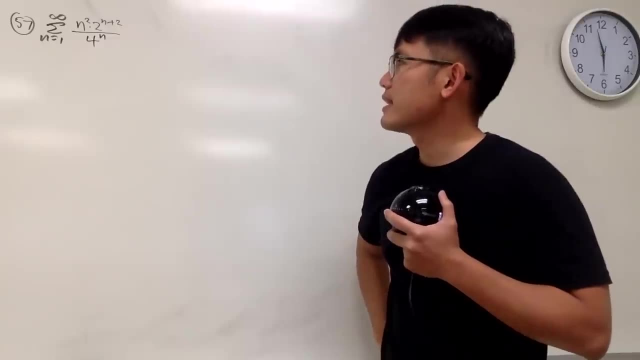 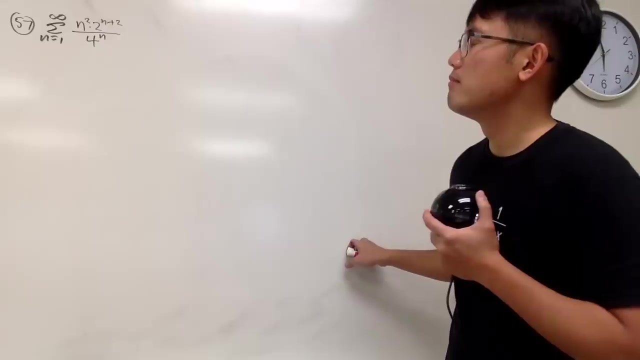 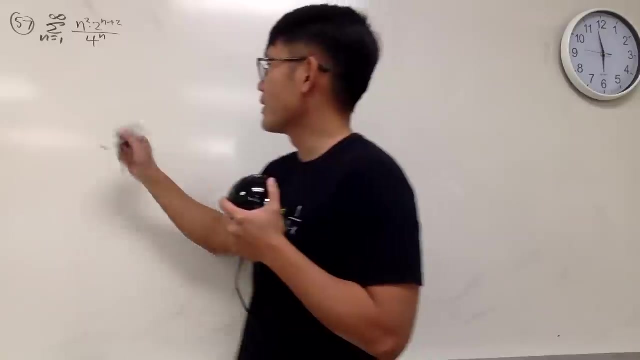 n plus 2 over 4 to the nth power, like that. Huh, God, Hmm. Let me just simplify the expression a little bit to make me feel better. Okay, To make us feel better. So notice that this right here. 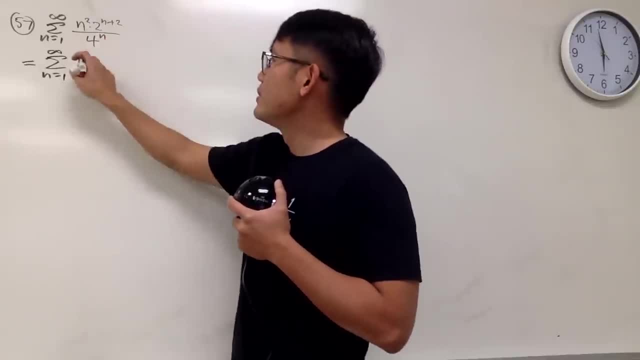 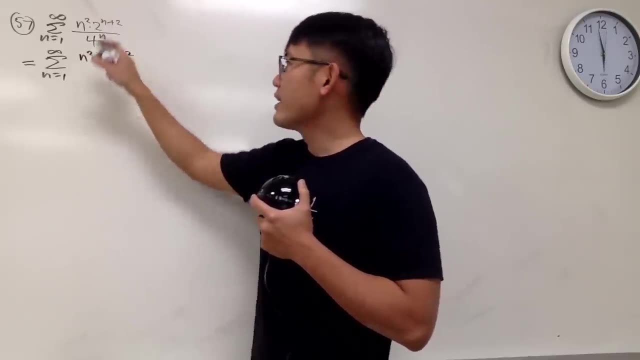 let's do some algebra right here. This is n equals 1 to infinity, and this is just n squared times. this is 2 to the n, and of course we can just say that's multiplied by 2 to the second power. and on the bottom, 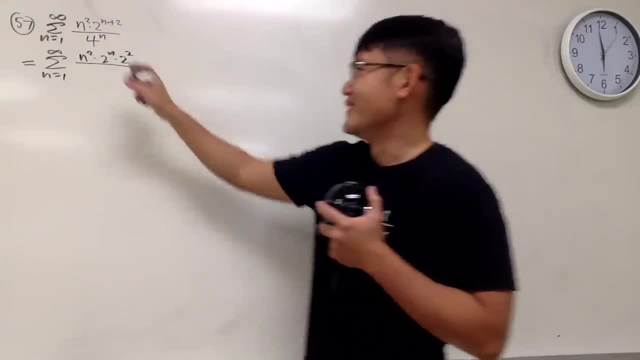 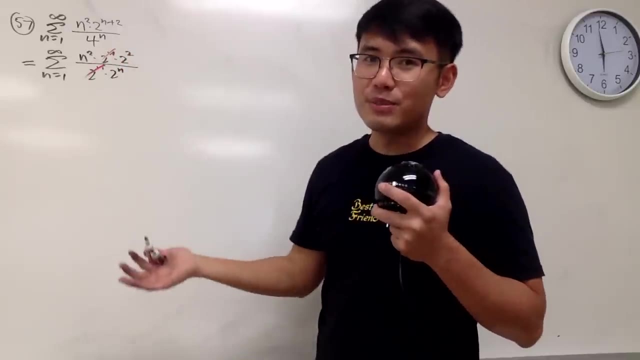 if you would like. 4 is the same as 2 to the n, so we can look at this as 2 to the n times 2 to the n, and the point is that I want to get rid of these two things. That's much better. 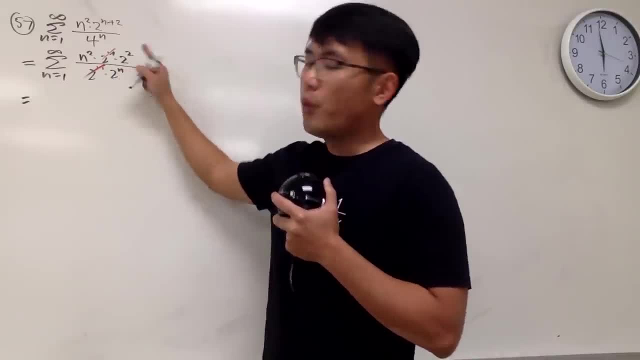 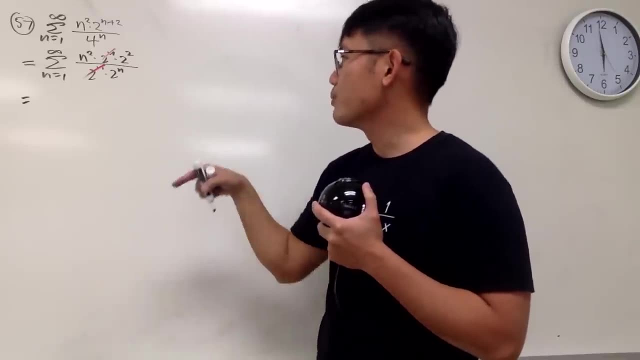 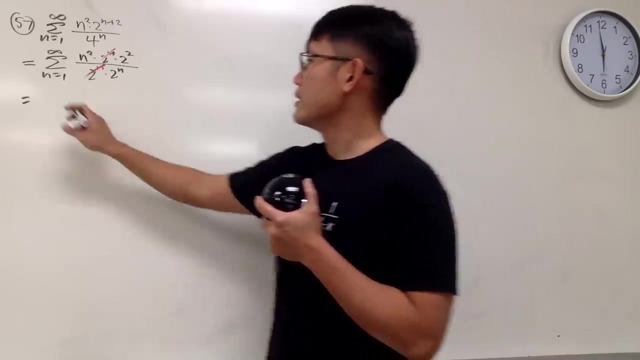 And in the end we see that this right here, we have 4 right here, right, And hmm, depends on how you want to do it, Maybe if you want to put a 4 in the front, or maybe we can do this. The sum as n goes from. 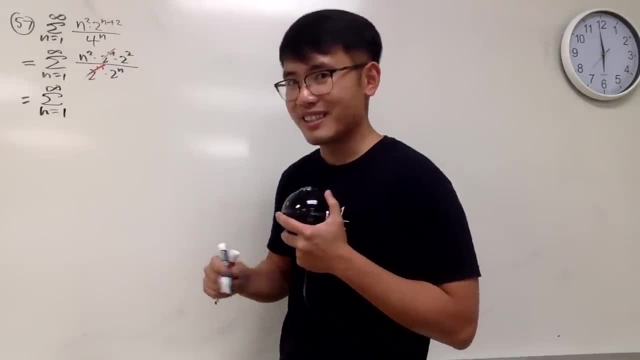 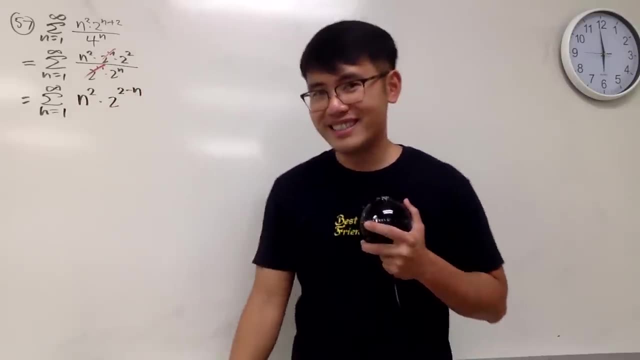 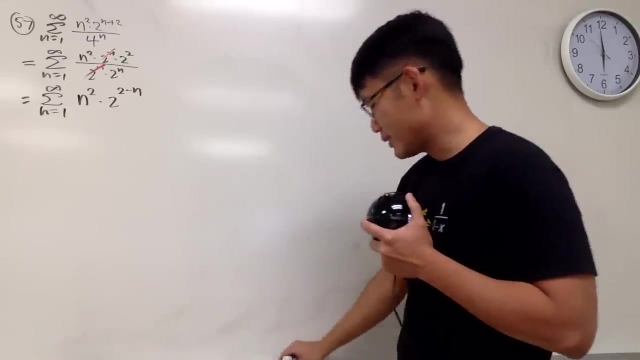 1 to infinity. maybe you will see a question like this on the test n squared times 2 to the 2 minus n power. this right here is weirder, but you have to remember the rule of exponents, of course. But anyway, the point is that 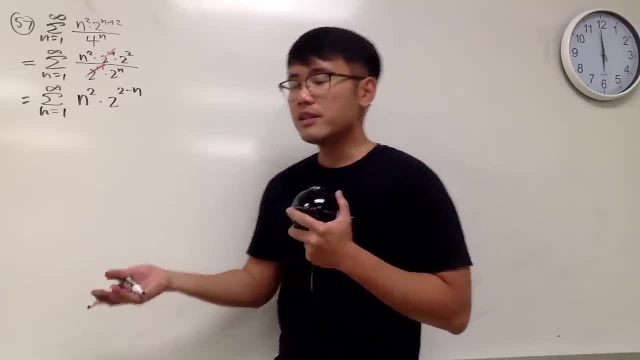 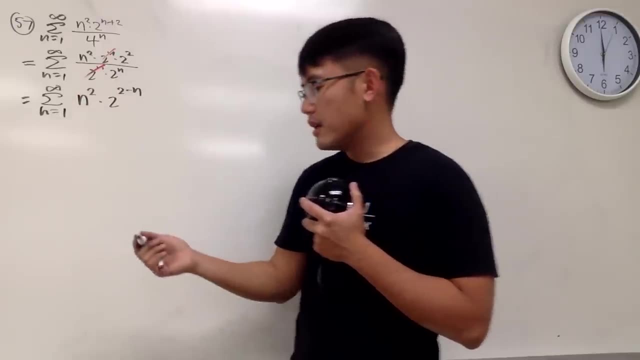 you have to just kind of play around with expression before you do anything, the usual thing. Here's the deal. let's do it by the ratio test and it's in the power, and this is not really geometric because of the n squared. The truth is: 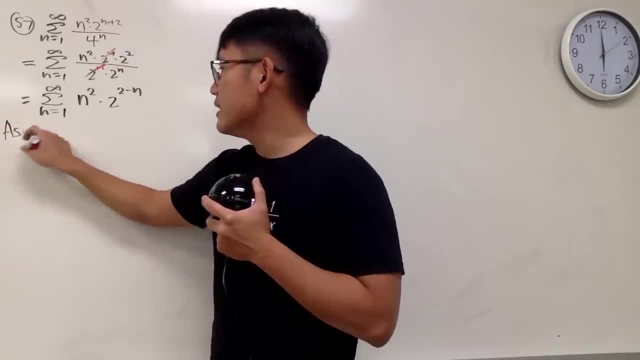 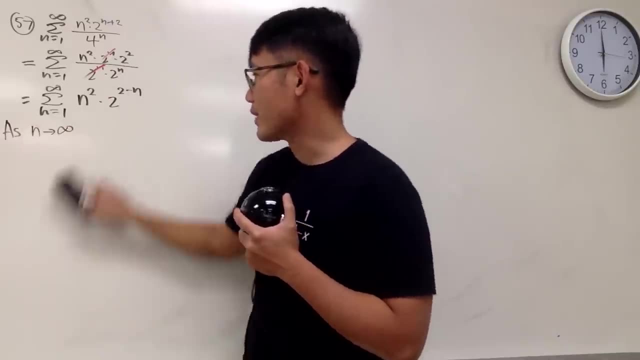 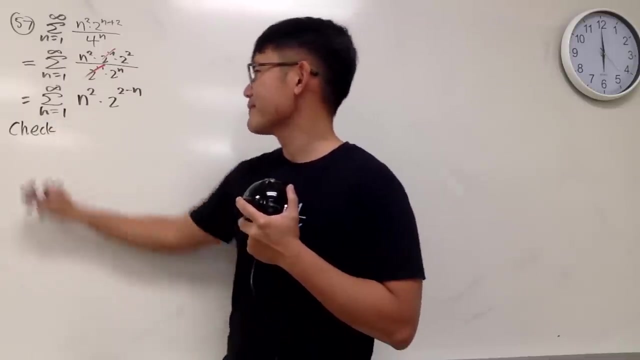 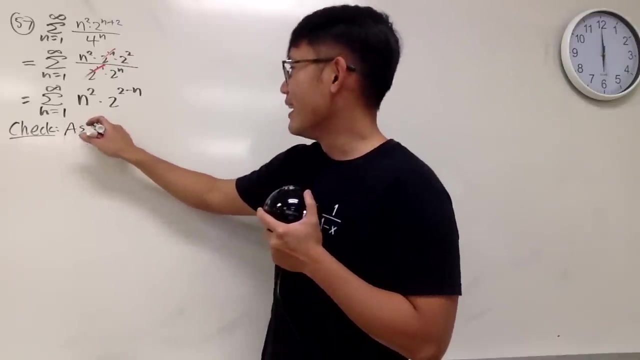 that it's not really geometric. but anyway, here's the deal: as n goes to infinity- and of course I forgot that word check, we check: as n goes to infinity, capital letter capital n. I mean capital capital A n goes to infinity. alright, first of all, all the 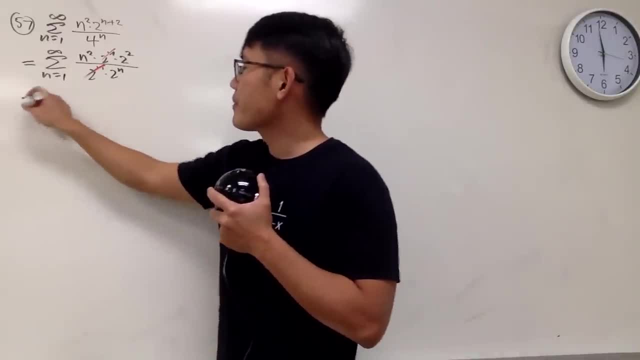 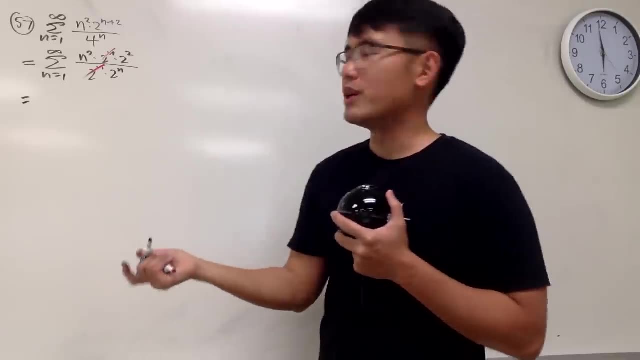 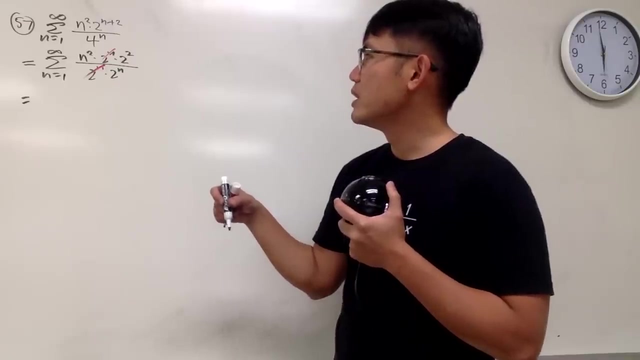 And in the end we see that this right here, we have 4 right here, right, And hmm, depends on how you want to do it. Maybe if you want to put a 4 in the front, or maybe we can do this. 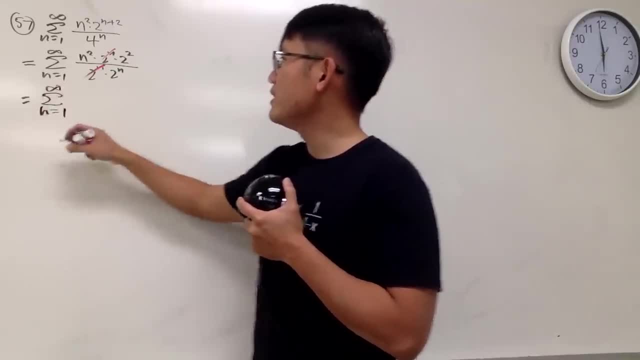 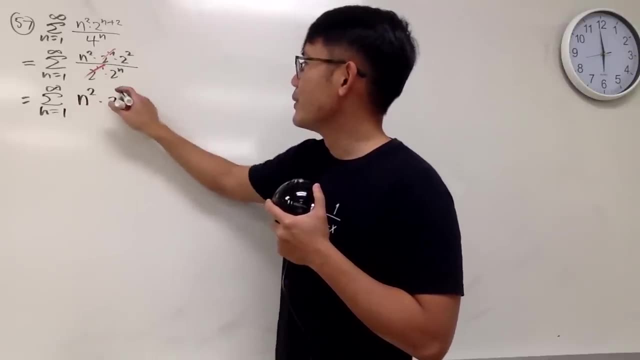 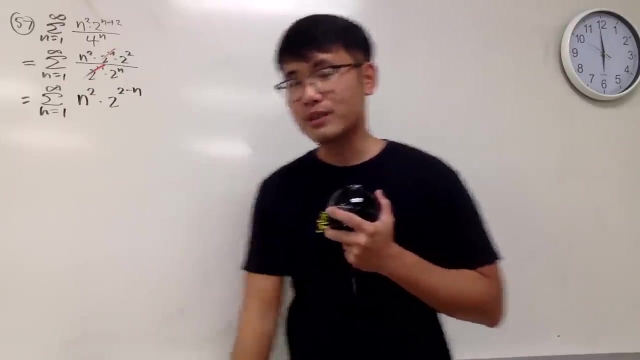 The sum as n goes from 1 to infinity. maybe you will see a question like this on the test n squared times 2 to the 2 minus n power. This right here is weirder, but you have to remember the rule of exponents. 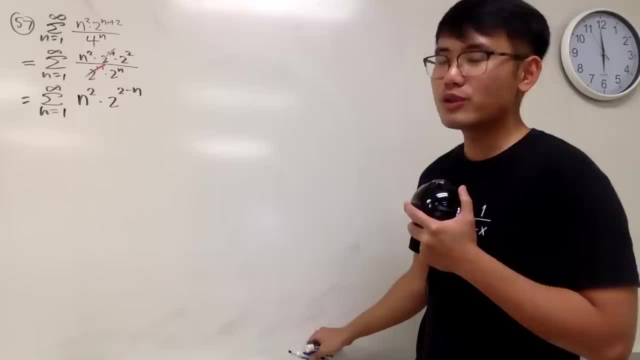 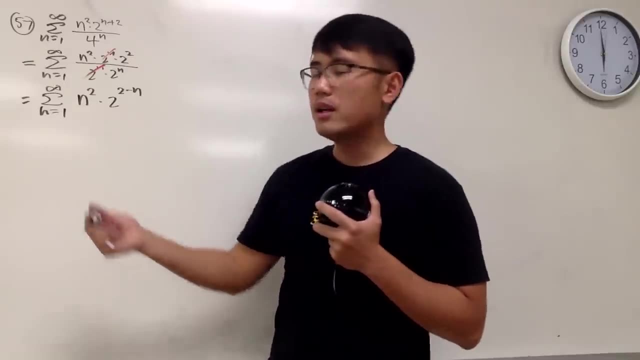 of course, But anyway, the point is that you have to just kind of play around with the expression before you do anything, the usual thing. Here's the deal. Let's do it by the ratio test, And it's in the power. 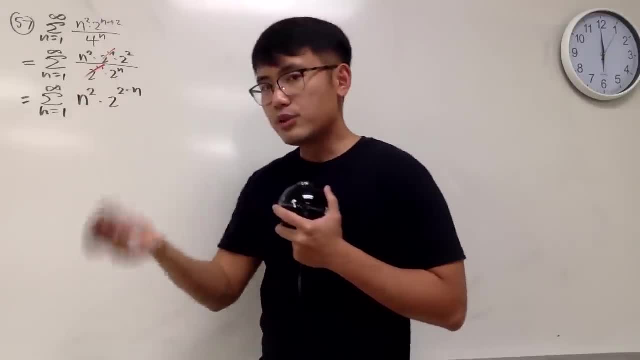 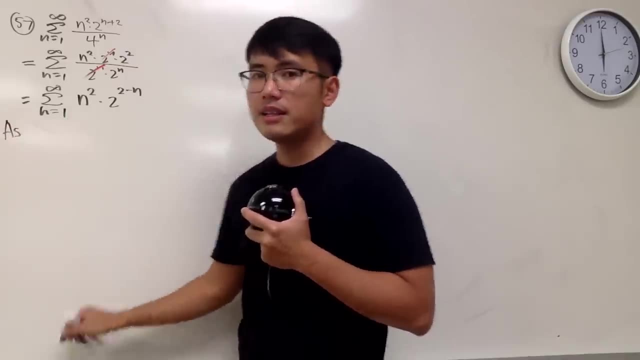 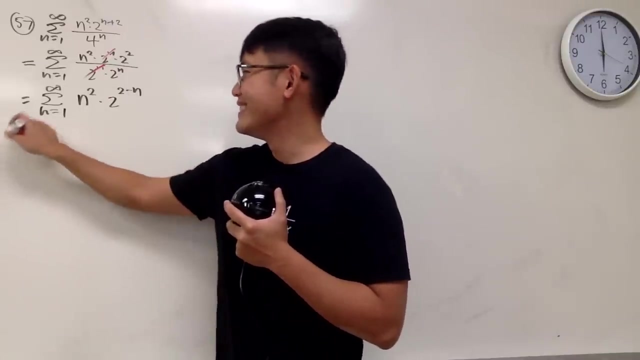 and this is not really geometric because of the n squared. The truth is it will converge. But anyway, here's the deal, As n goes to infinity. and of course- oh, I forgot the word check, We check, as n goes to infinity. 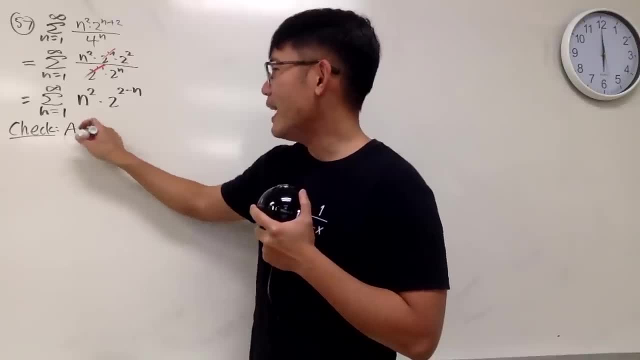 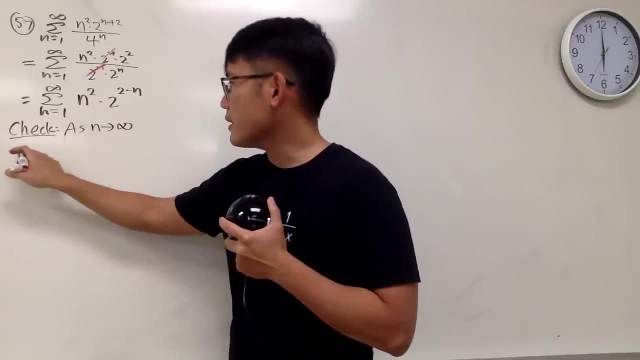 capital letter, capital n. I mean capital A. capital A n goes to infinity. All right, first of all I want to have all the well. take the absolute value first, And then all the m's become n plus 1,. 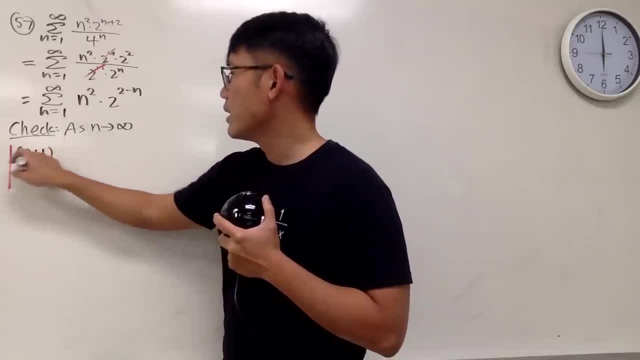 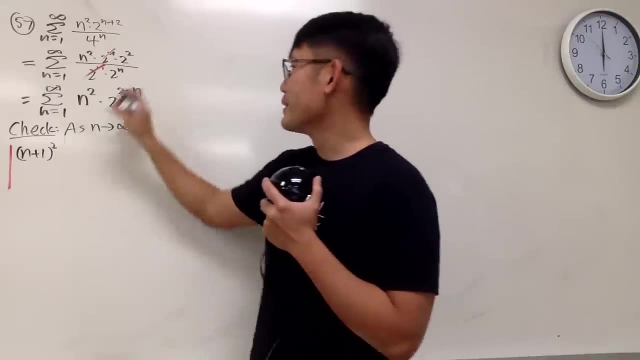 so we have this right here being n plus 1 squared, And of course you have to know this is the same as that. I just want to show you guys. this might be the question on the test, So I'll put this down right here. 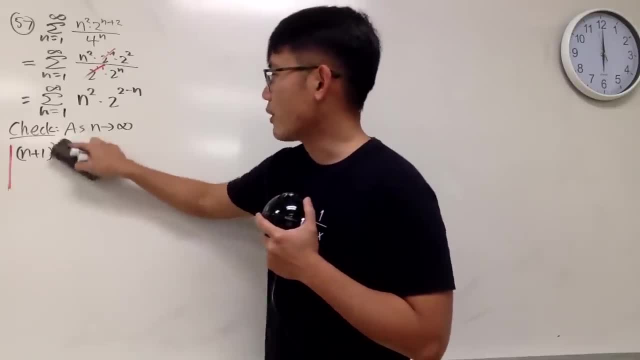 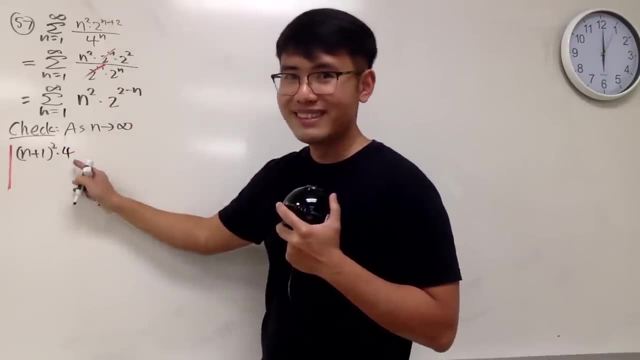 times 2 to the 2 to the 2 is 4,. come on right. This right here is, of course, 4.. That's 4, right. This right here is 4. Over 2, and we'll just put down n plus 1.. 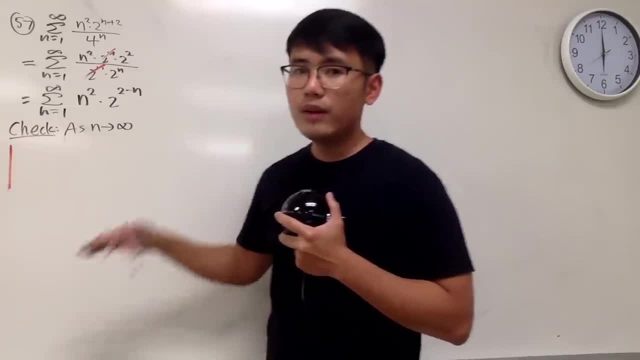 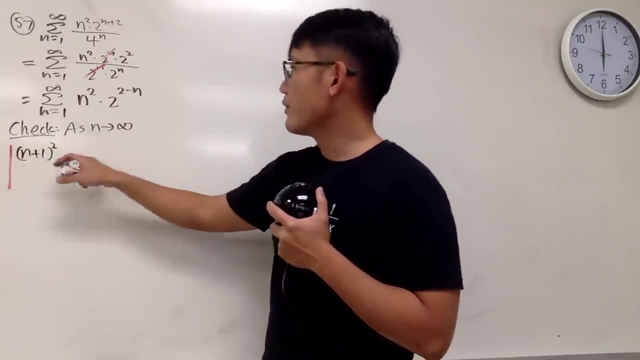 well, take the absolute value first, and then all the n's becomes n plus 1, so we have this right here, being n plus 1 squared, and of course you have to know this is the same as that. I just want to show you guys. this might be the question. 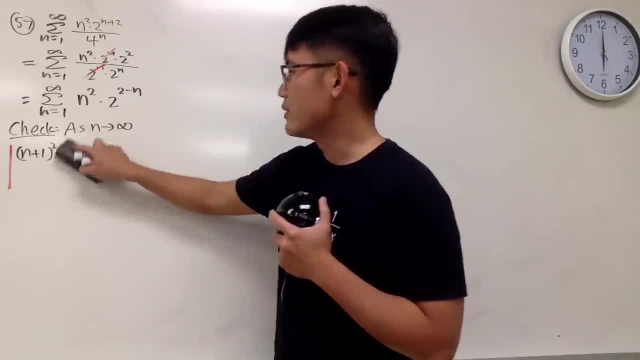 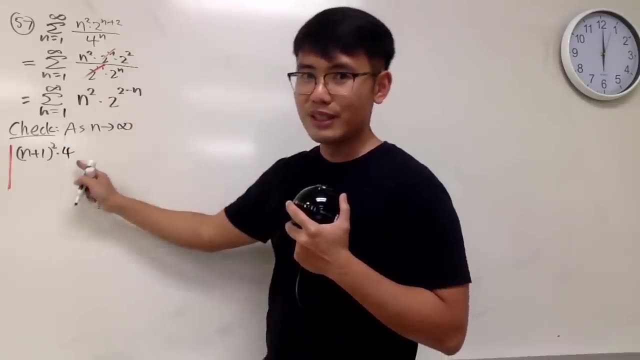 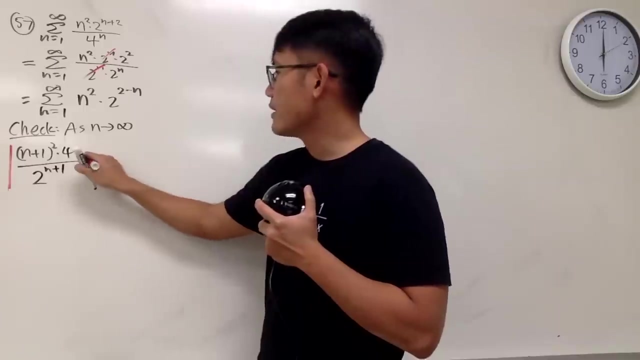 on the test. So I'll put this down right here. times 2 to the 2 to the 2 is 4. come on right. this right here is of course 4 over 2, and we'll just put down n plus 1, okay. 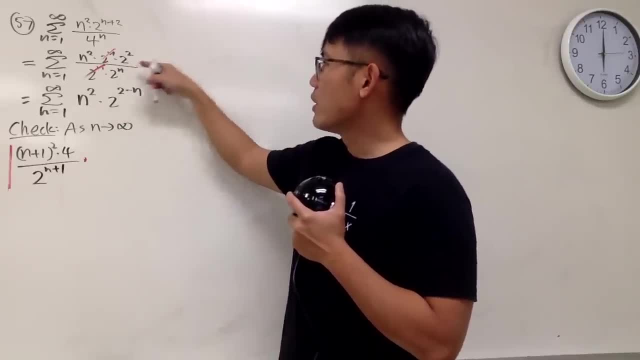 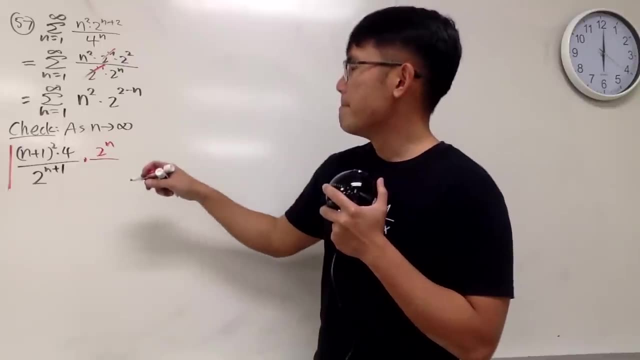 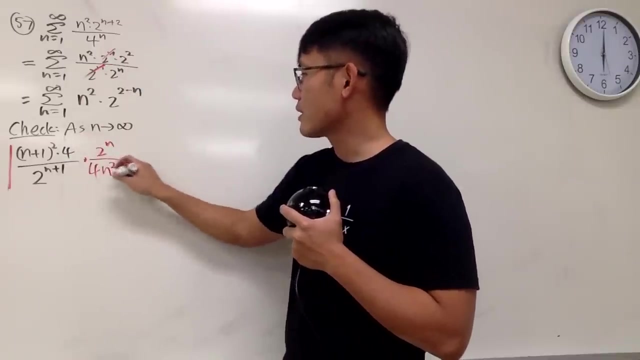 times the reciprocal. so I will look at 2 to the n first on the top, and we do that over this and that. so let's put a 4 first, like seriously, what the hell? just write down as a 4 and then n squared like this: 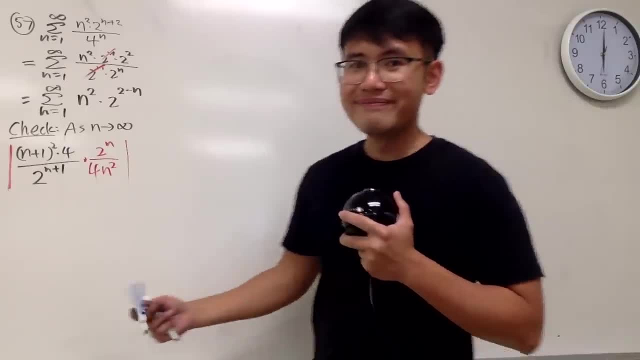 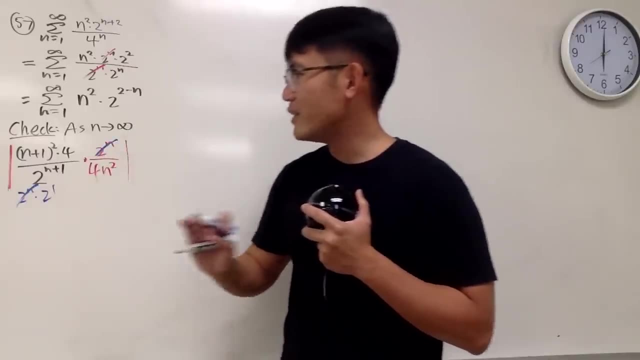 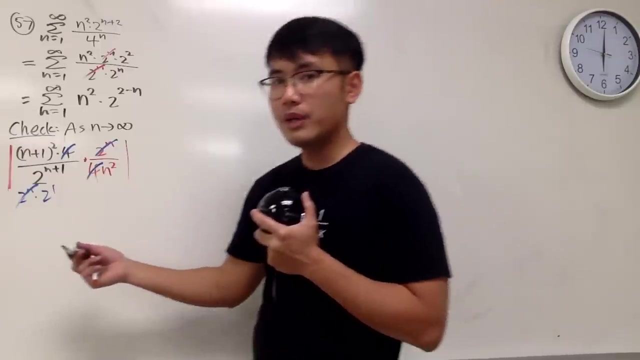 okay, now, here is the deal. this, right here we can do what. yeah, 2 to the n times, 2 to the first, cancel, cancel, very, very nice, let's carry the 4 already, seriously, okay, now let's do the algebra. and when we do the algebra, 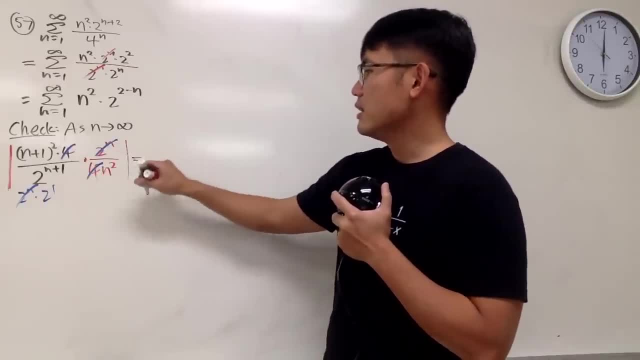 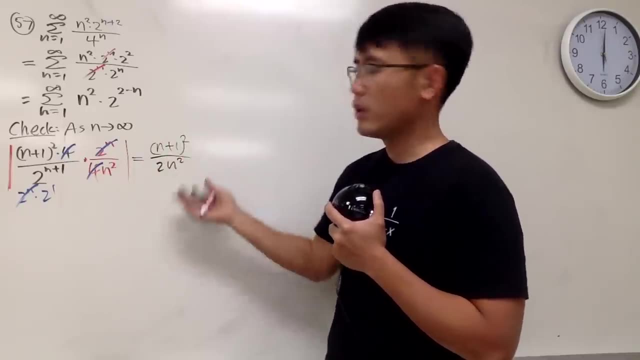 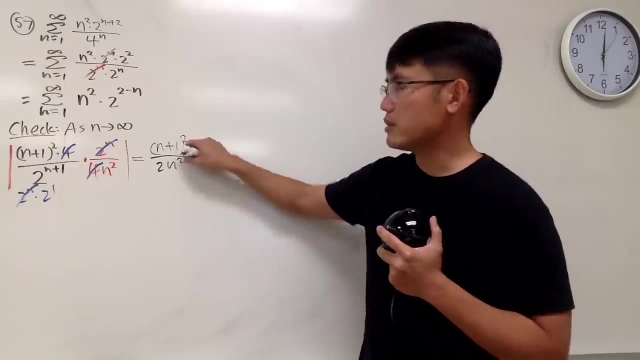 we will see that this right here is equal to the top. everything is positive again. it's just n plus 1 squared over 2, n squared like this. this time again, the powers right here. that's finite. so truth is this right here is just going to be. 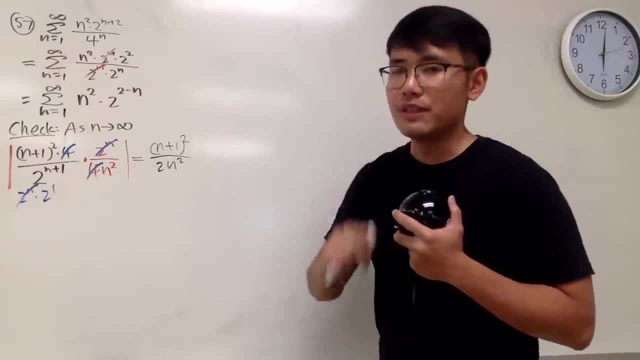 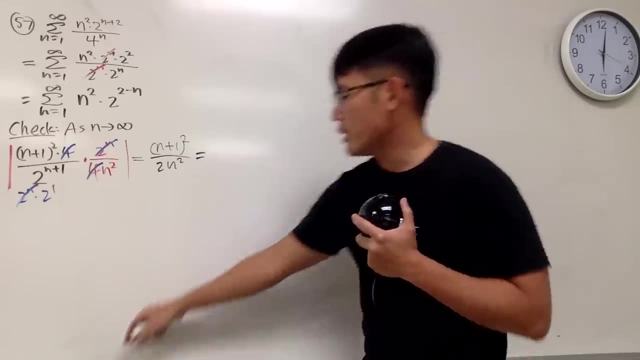 1 and then you have the 2, so altogether it's 1 half. but if this is n, this is n. you have to use the fact anyway, just to show you this right here, we can actually multiply the whole. and let me, let me just do it right here. 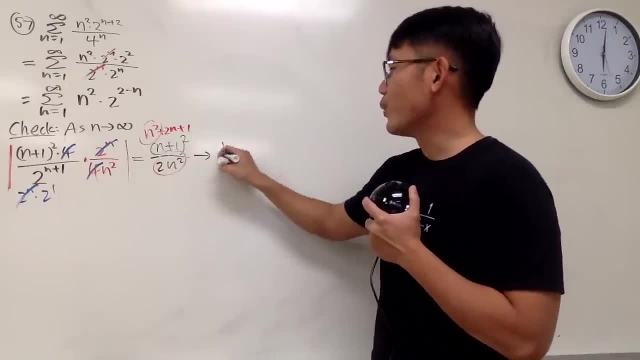 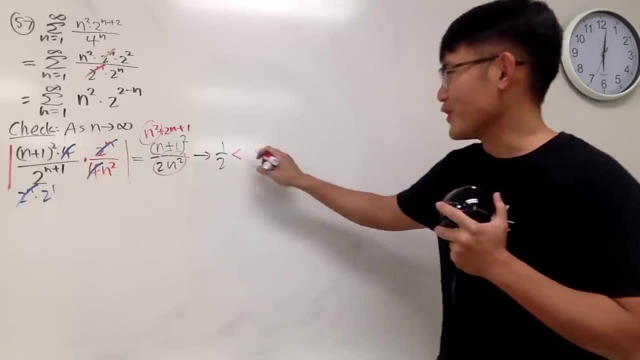 this is the same as saying: n squared plus 2n plus 1, take this, take that, so this. right here we are doing the ratio test, okay, okay, okay, hopefully you guys didn't see it. this right here is less than 1, so we can draw a conclusion. 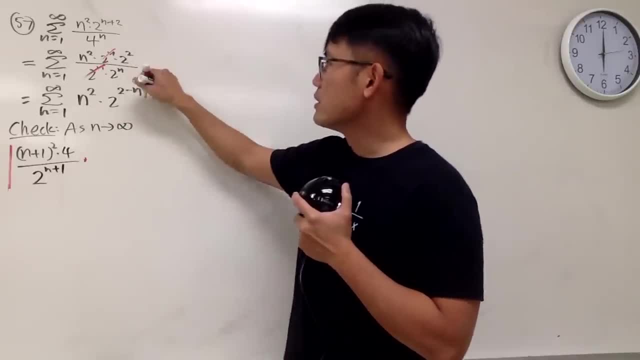 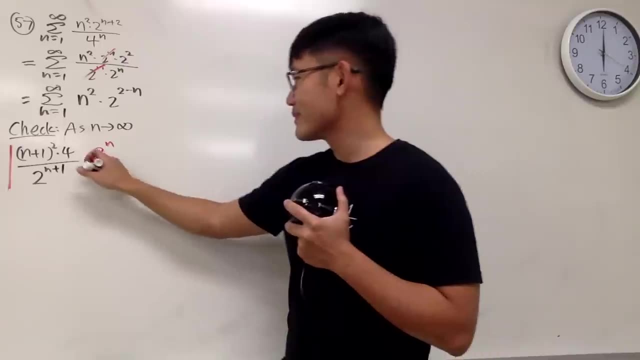 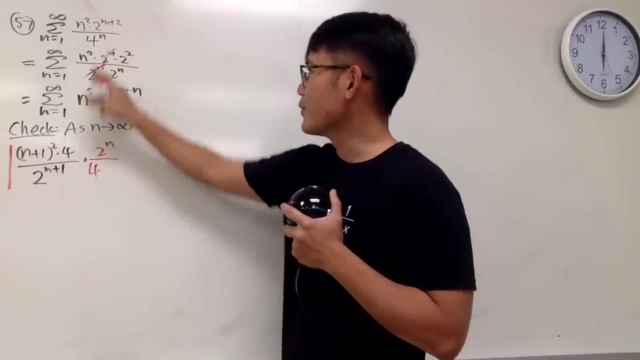 Okay, times the reciprocal, so I will look at 2 to the nth first on the top and we do that over this and that, So let's put a 4 first. Like seriously, what the hell just write down as a 4,. 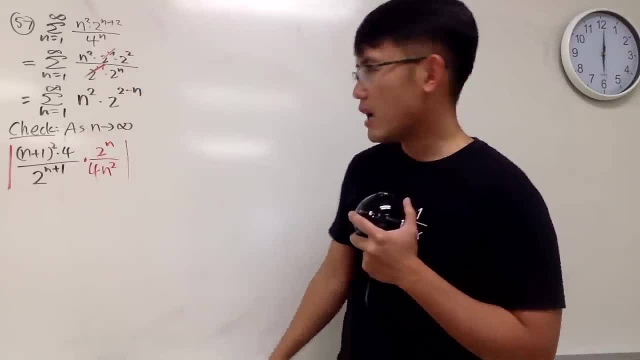 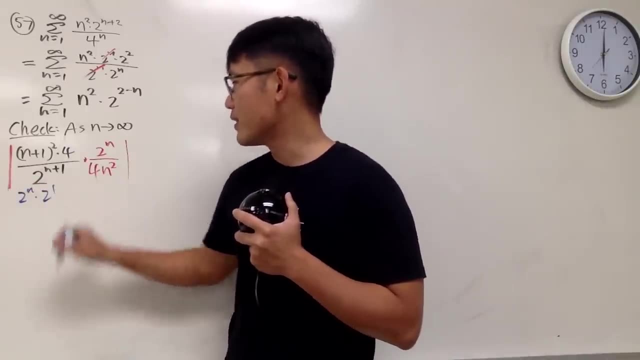 and then n squared like this: Okay, Now, here is the deal. This right here, can we, we can do what? Yeah, 2 to the n times, 2 to the 1st, Cancel, cancel, Very, very nice. 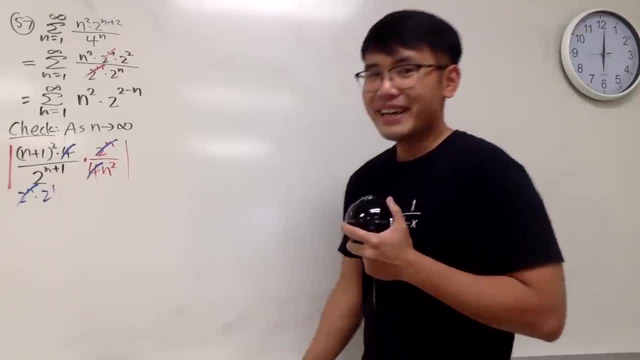 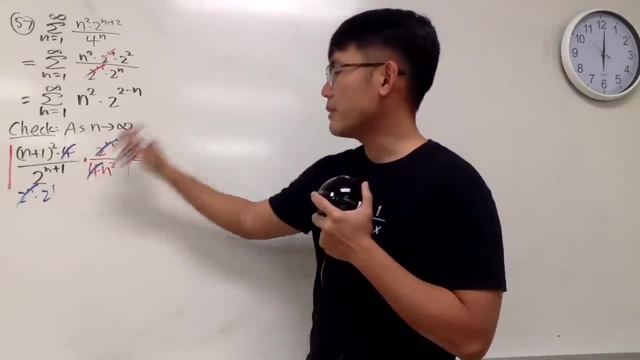 Let's carry the 4 already seriously. Okay, now let's do the algebra. and when we do the algebra we will see that this right here is equal to the top. everything's positive again. It's just n plus 1,. 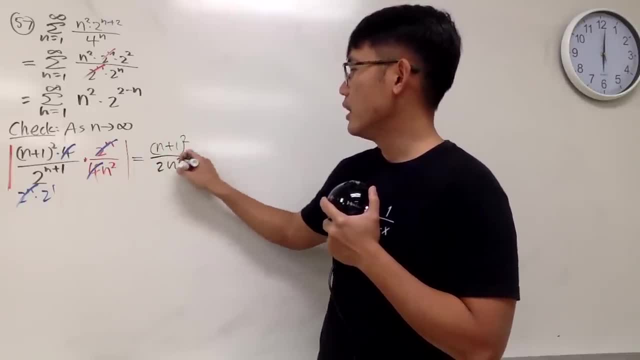 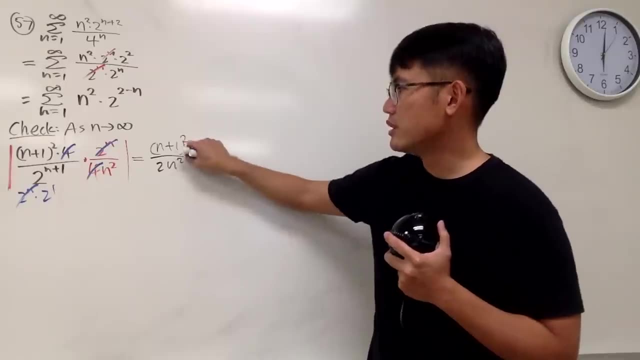 squared over 2, n squared like this. This time again, the powers right here. that's finite. so truth is this: right here is just going to be 1, and then you have the 2,, so altogether it's 1 half. 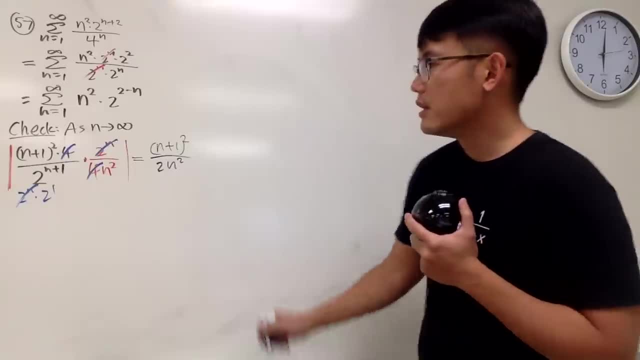 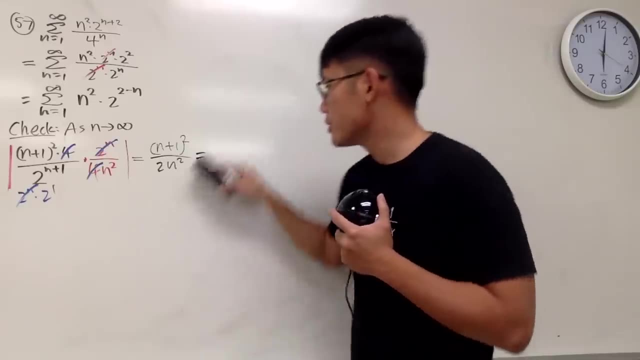 But if this is n, this is n. you have to use the fact. Anyway, just to show you this right here, we can actually multiply the whole, and let me, let me just do it right here. This is the same as saying: 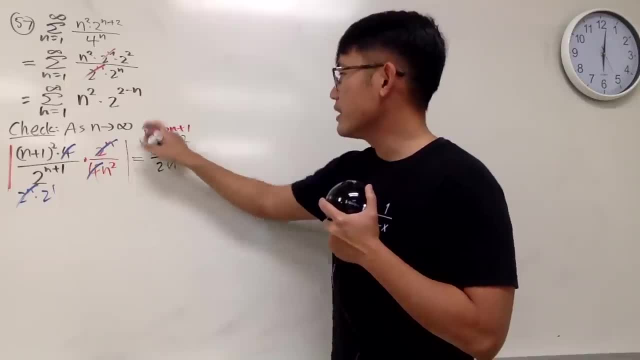 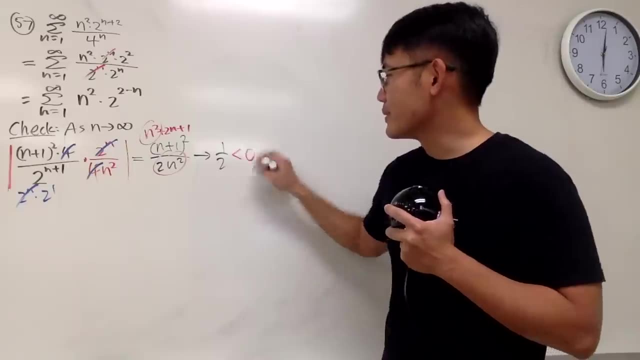 n squared plus 2n plus 1, take this, take that, so you get 1 half Done, And the beauty is that this, right here we are doing the ratio test, Okay, Okay, okay, hopefully you guys didn't see it. 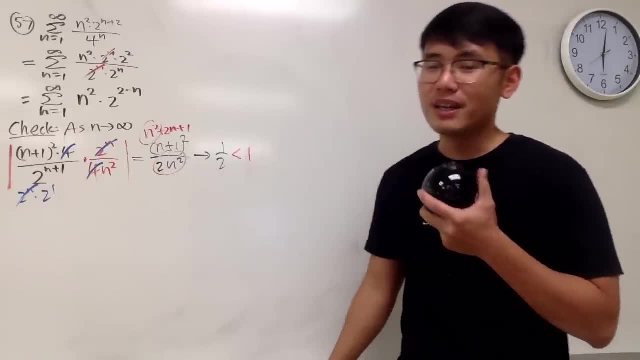 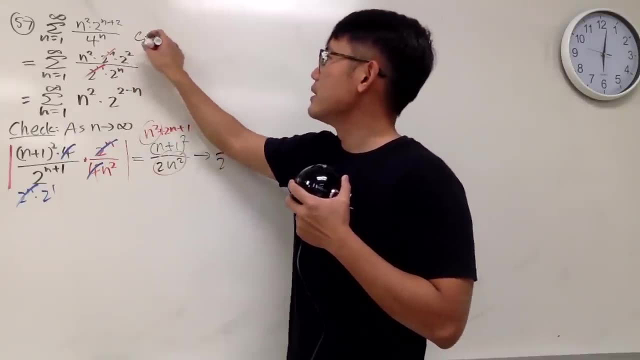 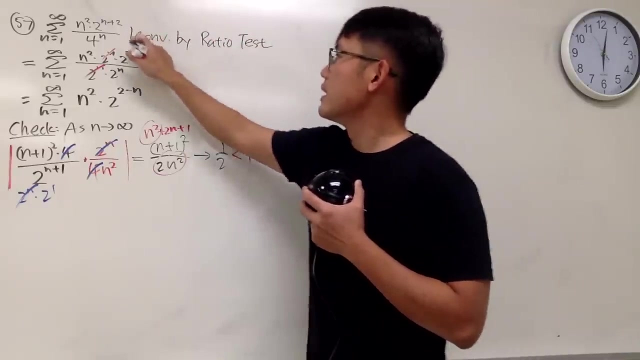 This right here is less than 1, so we can draw a conclusion because again, we're using the ratio test, Very, very nice. So this right here converges by the ratio test, Like that. Okay, Very good. 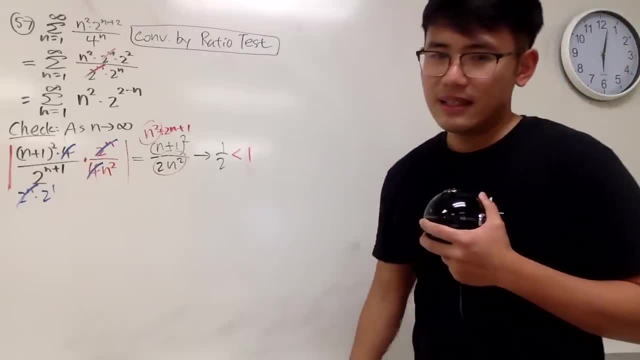 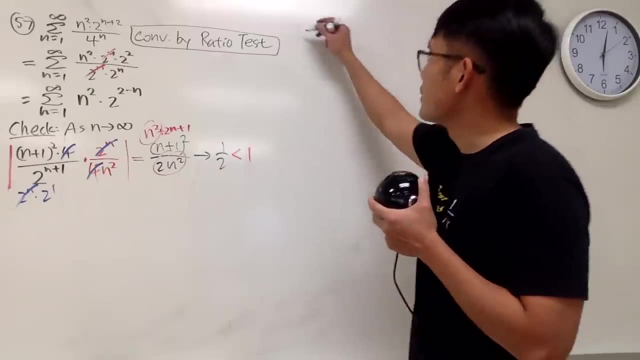 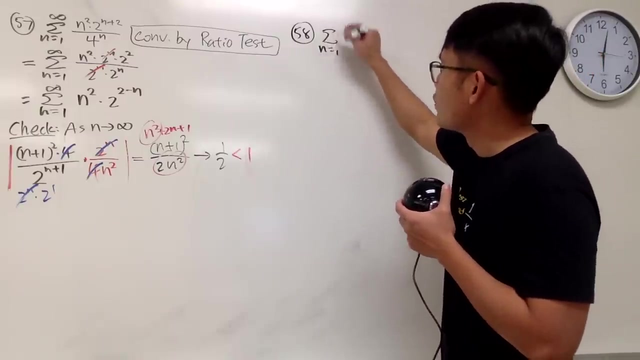 Now 58. Hmm, Okay, Let me put it down right here, Number 58.. Right here, Here we go. Take the sum as n goes from 1 to infinity parentheses, the nth root of 2,. 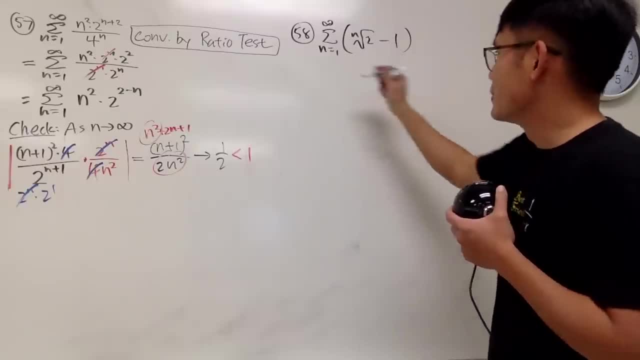 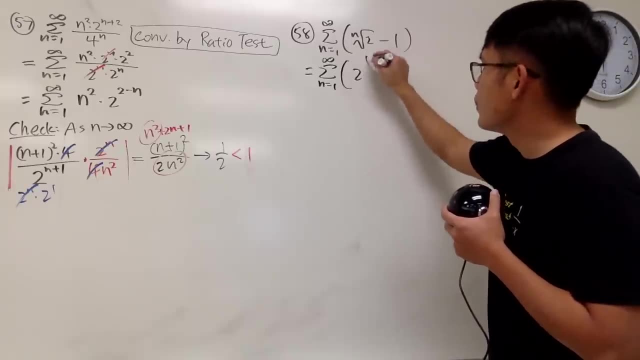 minus 1.. Oh God, Okay, let's look, let's study, let's make this study better. Infinity is right here and blah, blah, blah. This right here is 2 to the 1 over n minus 1.. 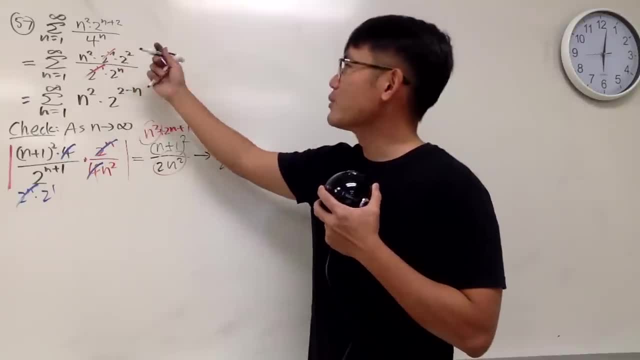 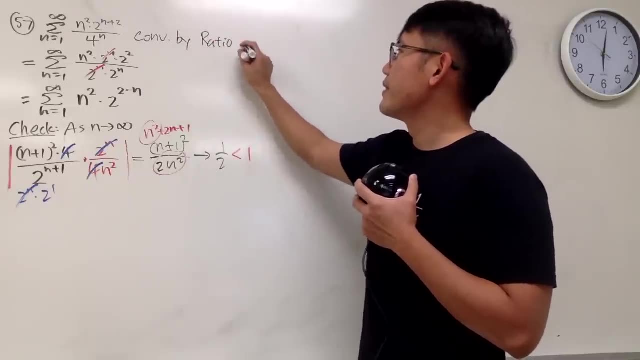 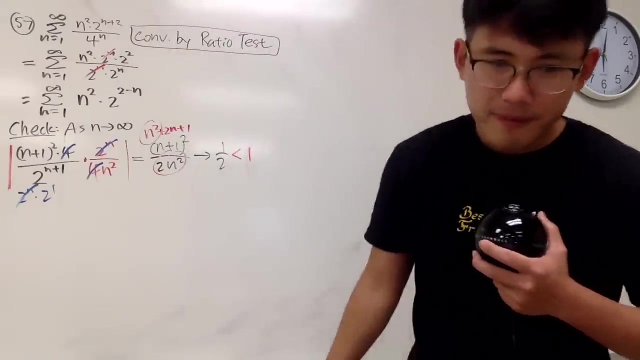 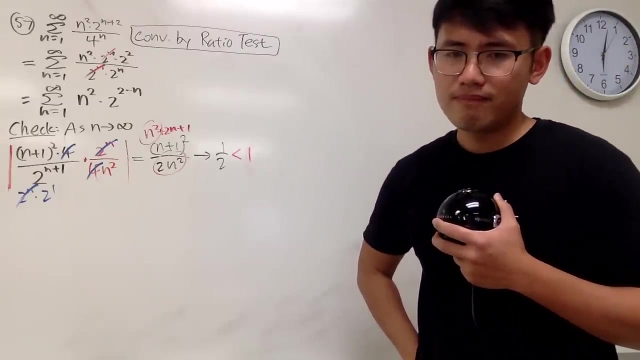 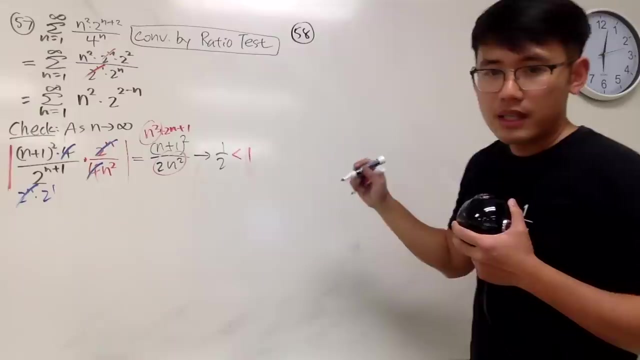 because again we are using the ratio test, very, very nice. so this right here converges by the ratio test, like that right. very good, now 58. hmm, okay, let me put it down right here number 58. right here, here we go. take the sum as n goes from 1 to infinity. 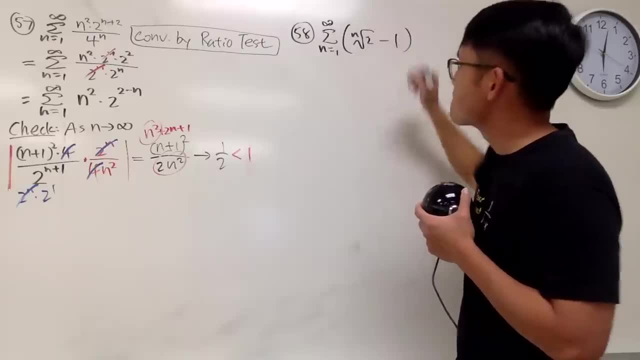 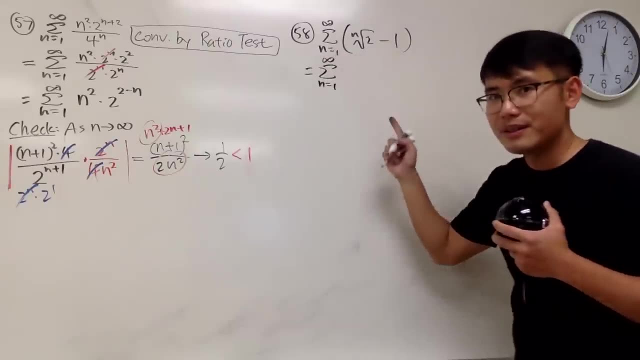 parentheses, the nth root of 2 minus 1. oh god, okay, let's look, let's study, let's make this study better. infinity right here, and blah, blah, blah. this right here is 2 to the 1 over n minus 1. d help, kind of. 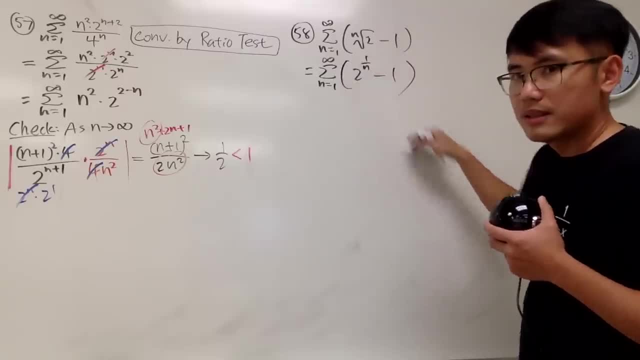 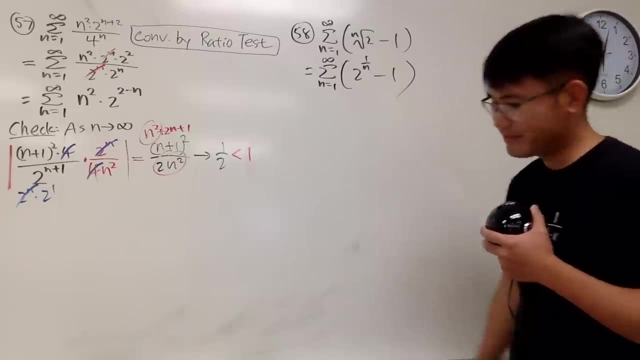 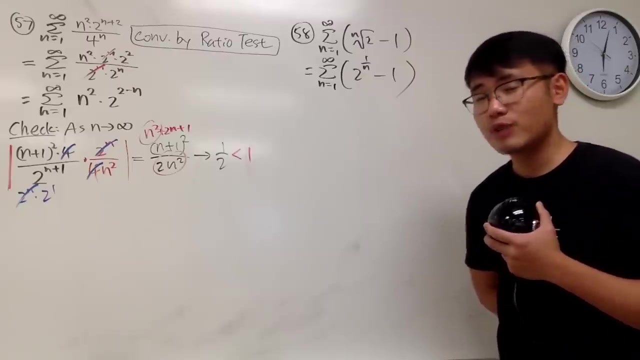 okay, if you take the uh limit test right test for divergence, you put infinity here, 2 to the 0th power pretty much is 1, 1 minus 1. oh man well, the test for divergence didn't work, but it's okay, let's try to do. 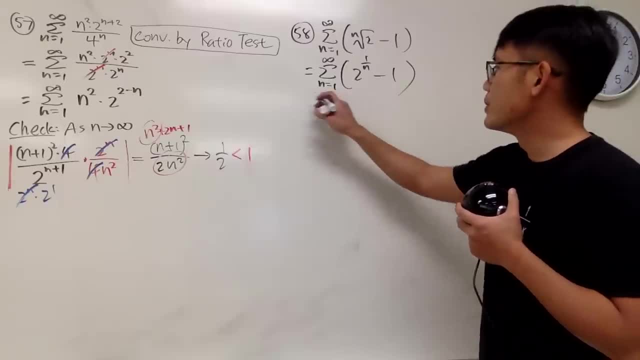 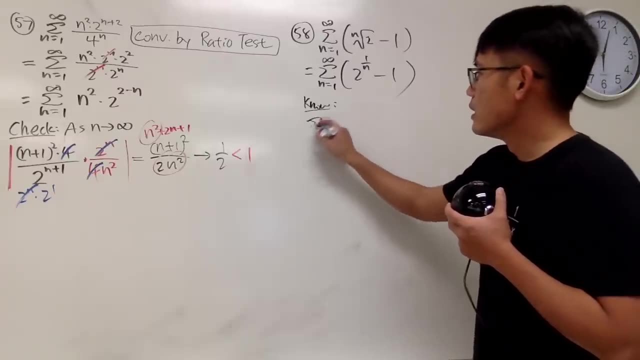 it's like comparison test. so again here, let's do the following. let's put down what we know, and it seems that we know- about 1 over n. I will just say the sum as n goes from 1 to infinity. 1 over n, right here. 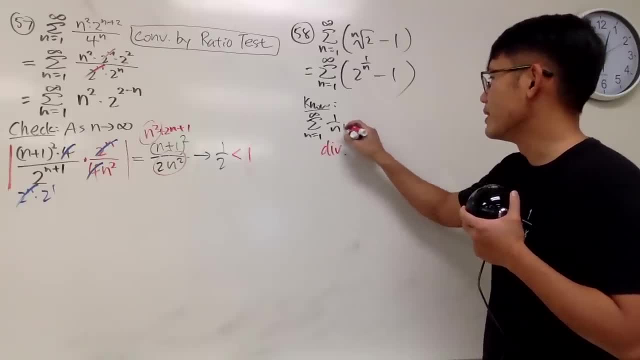 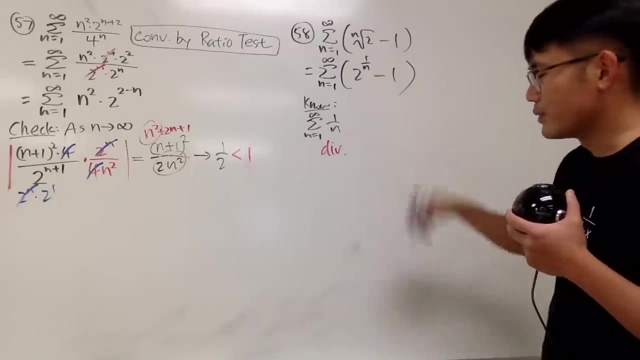 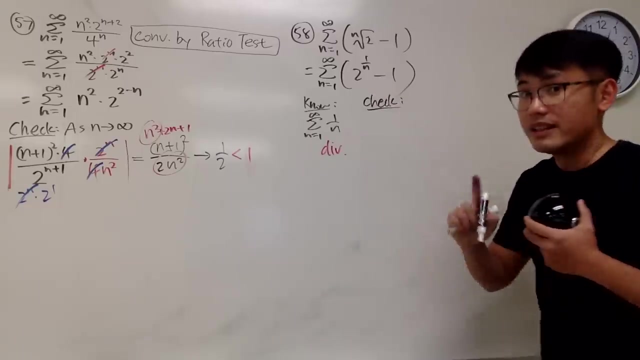 this right here diverges. I am not going to write down, still write down. this is this right here is diverges. you don't have to write down the reason, it's just really easy. this right here diverges. and now we are going to check the limit. 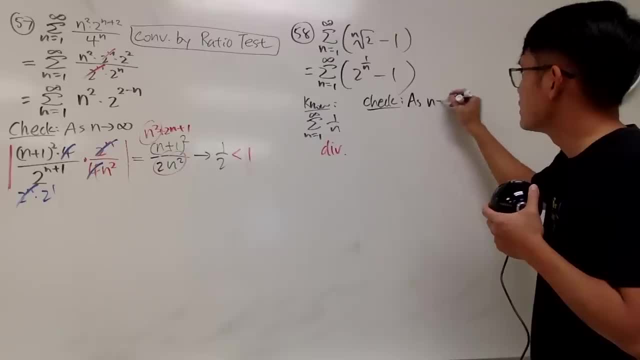 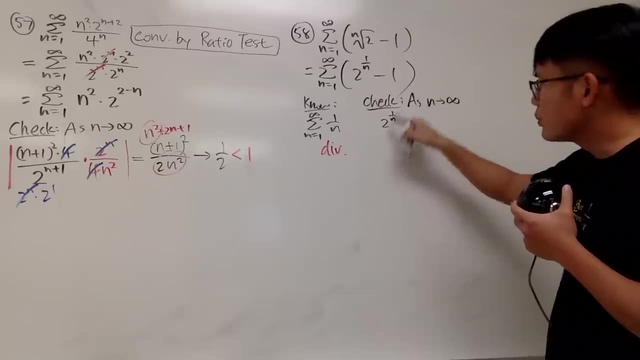 when, well, just put down, s? n goes to infinity. put the one that you want to do on the top, which is 1 over 2, to the 1 over sorry, 2 to the 1 over n, minus 1 over the one that we are trying to get. 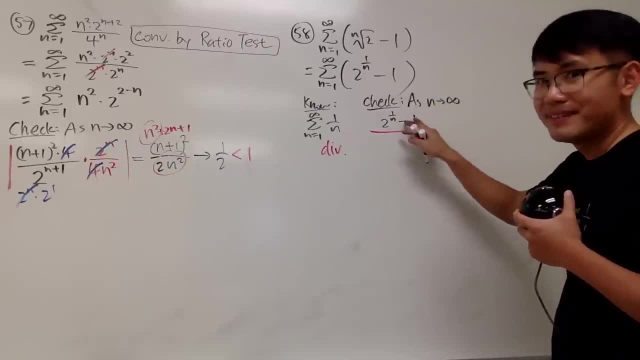 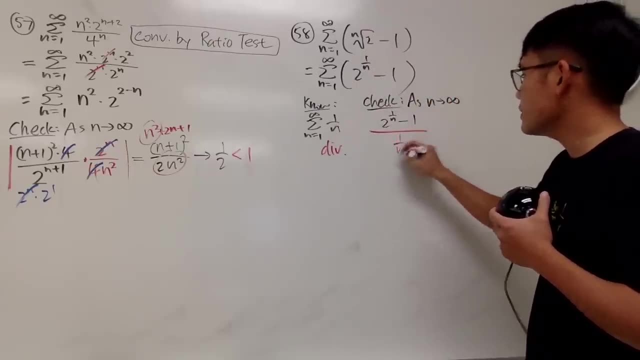 sorry, put the one that we we are trying to get on the top and then put the one that we know much better right here, just the that's called a? n power, not b? n power, right? all that? the good thing is that this is 0 over 0 situation. 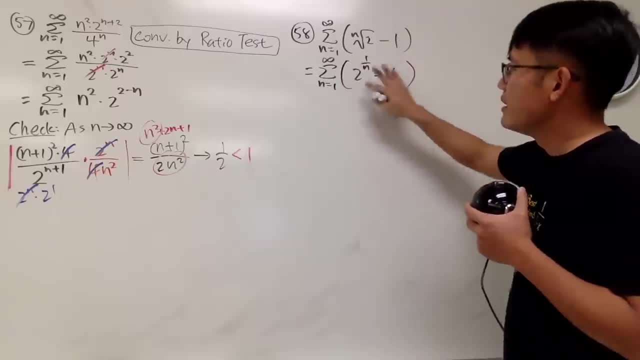 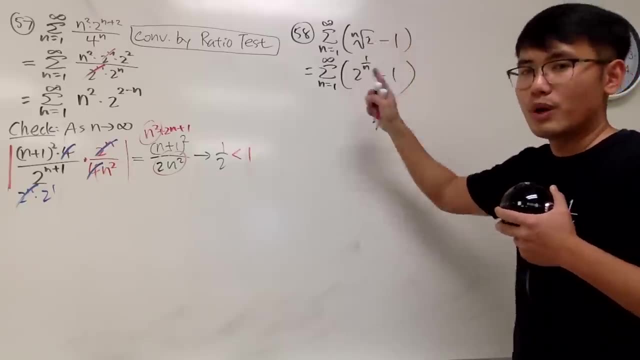 Did it help. Kind of Okay. If you take the uh limit test test for divergence, you put infinity here. 2 to the 0th, power pretty much is 1.. 1 minus 1 is: 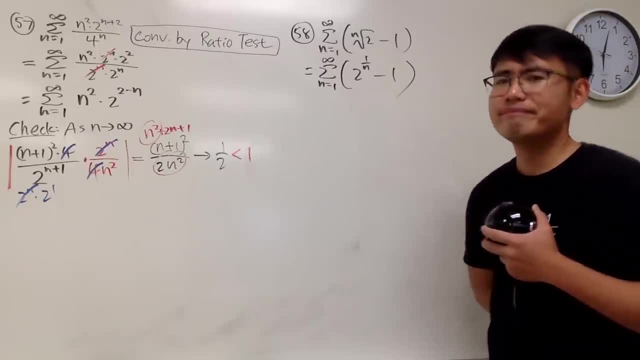 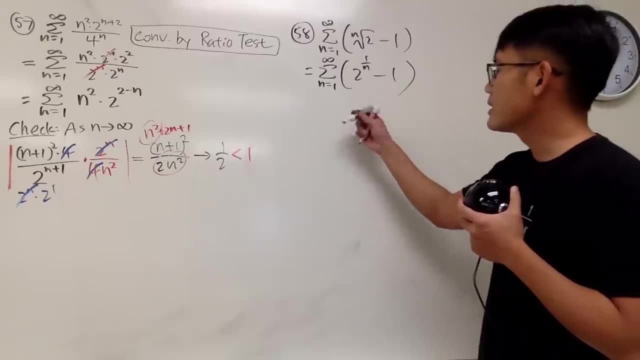 oh, man, Tsk. Well, the test for divergence didn't work, but it's okay, Let's try to do. it's like comparison test. So again here, let's do the following: Let's put down what we know. 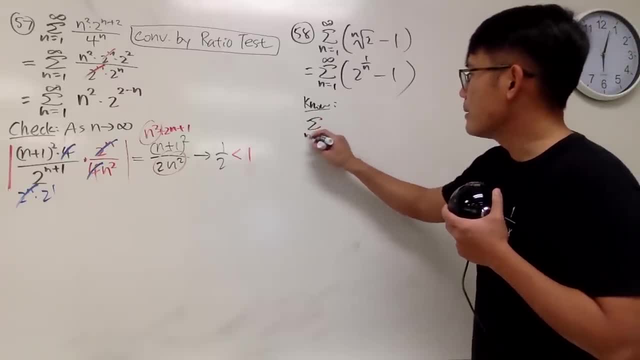 and it seems that we know about 1 over n pretty well, So I will just say the sum as n goes from 1 to infinity. 1 over n, right here. this right here diverges, I am not going to write down. 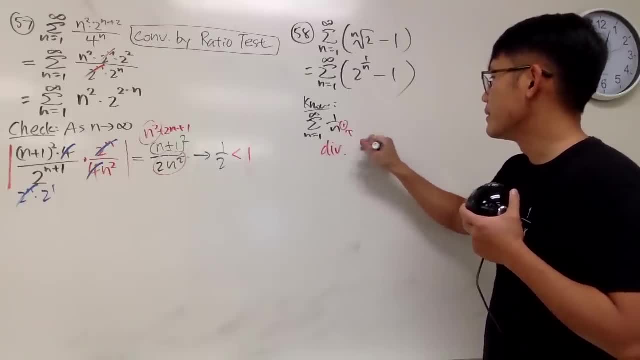 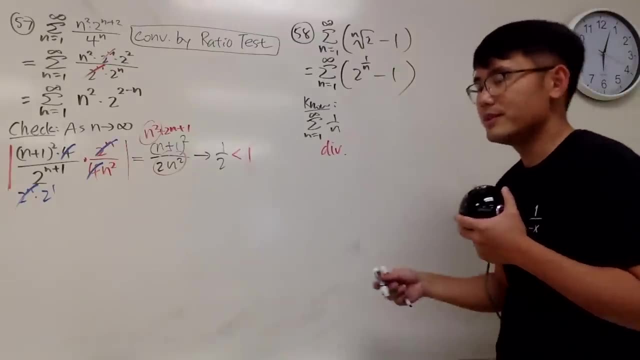 still still write down. This is. this right here is diverges. You don't have to write down the reason, it's just really easy. This right here diverges, and now we are going to check the limit when. 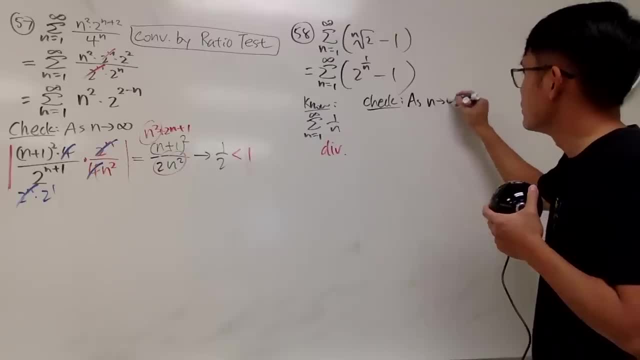 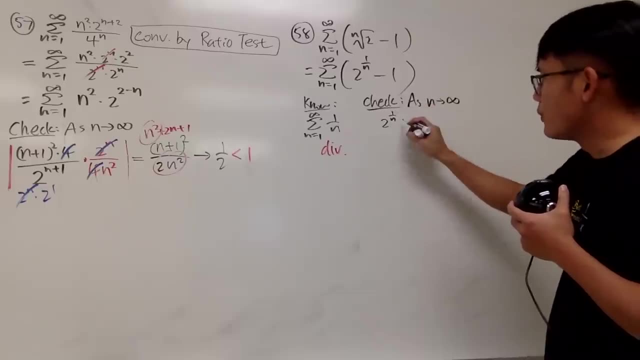 well, I'll just put down: s n goes to infinity. Put the one that you want to do on the top, which is 1 over 2, to the 1 over sorry, 2 to the 1 over n. 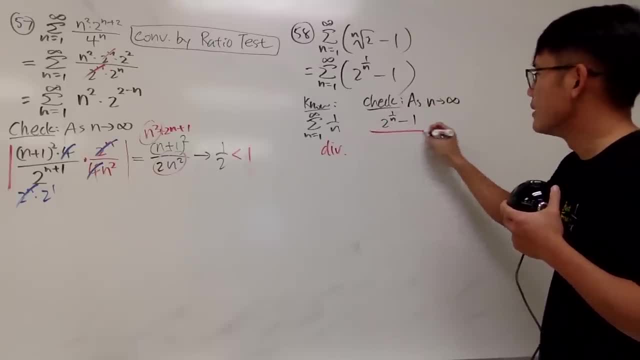 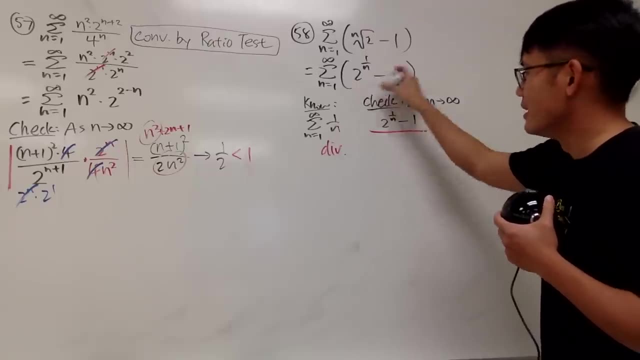 minus 1.. Over the one that we are trying to get, sorry, put the one that we we are trying to get on the top and then put the one that we know much better right here. just the that's called a n part. 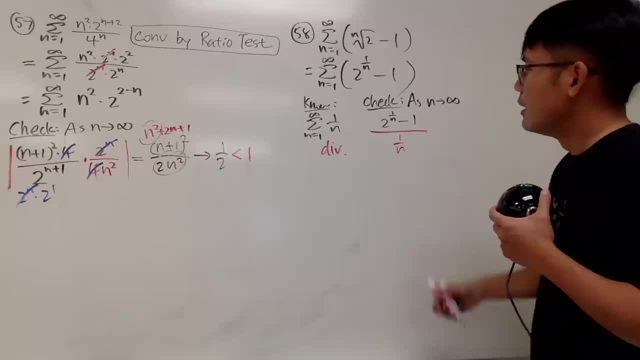 and not b? n part right, So we don't have to do all that. The good thing is that this is a 0 over 0 situation, but the bad thing is that we have to use Lapito's rule. 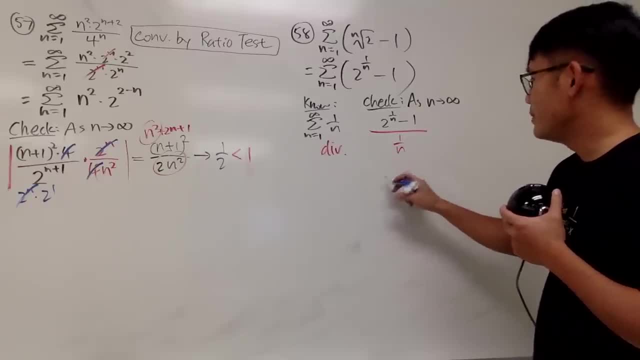 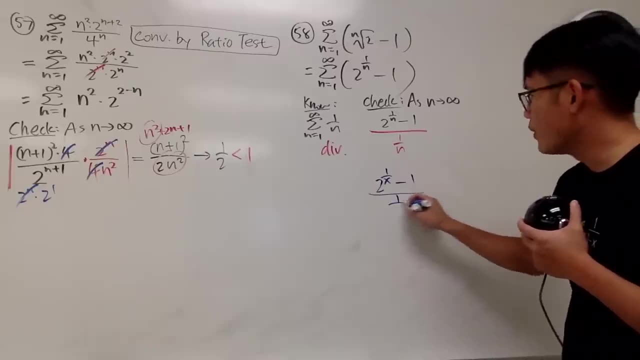 And the worst thing is that we have to change that to x. So let me just write this down: 1 over, I mean 2 over 2 to the 1 over x power minus 1, over 1 over x. 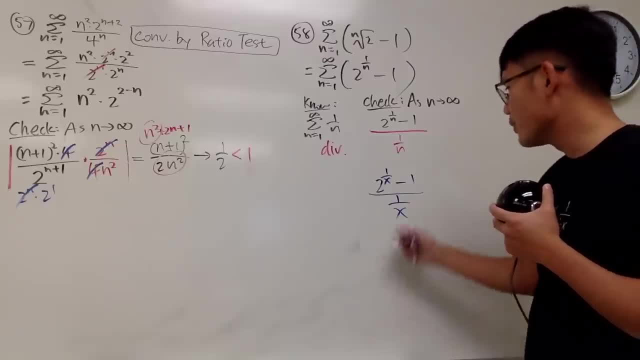 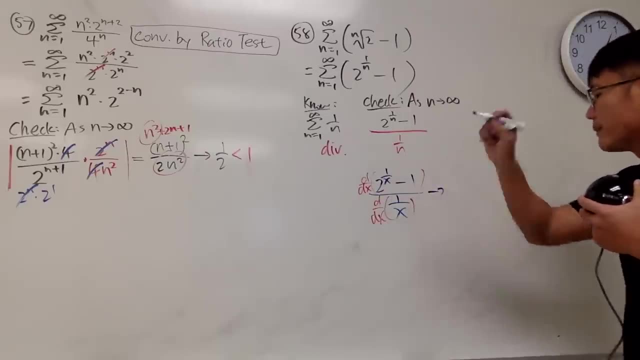 as x goes to infinity. Right here I'm just going to do the Lapito's rule d, dx, d dx and see what happens. This right here becomes: well, here we get negative 1 over x squared. 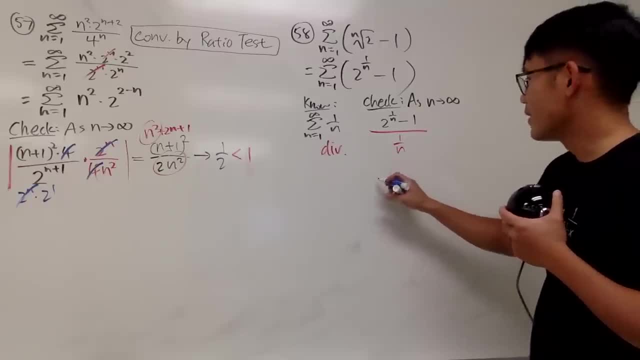 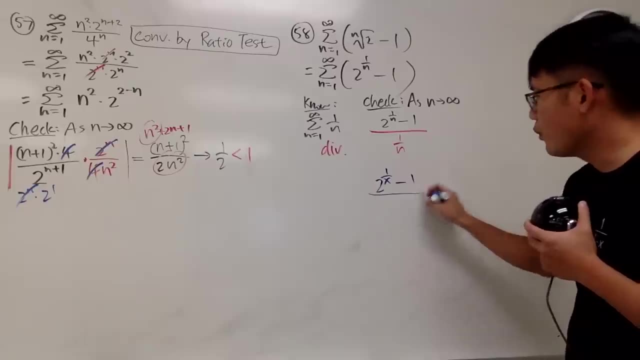 but the bad thing is that we have to use Lapito's rule and the worst thing is that let me just write this down: 1 over I mean 2 over 2 to the 1 over x power minus 1 over 1 over x. 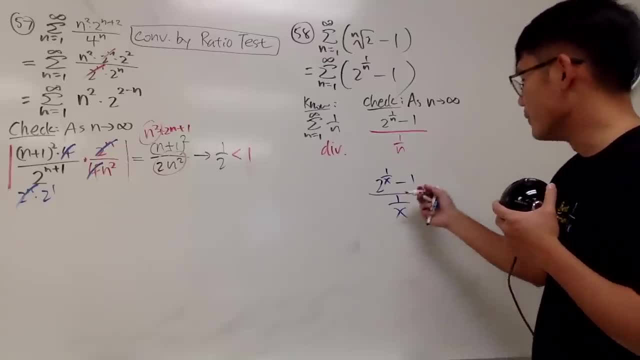 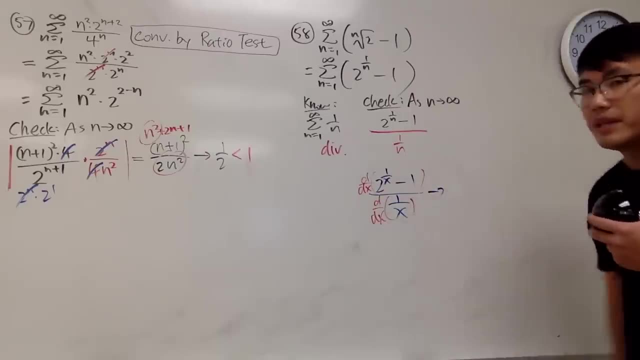 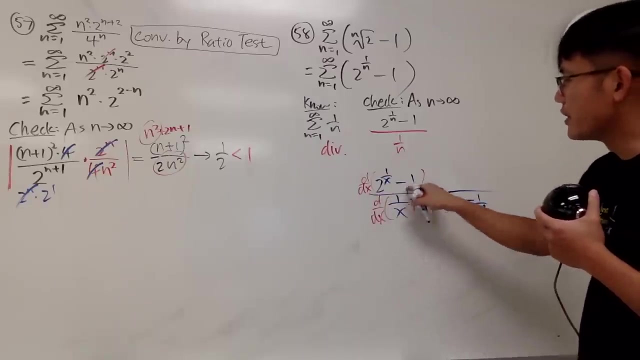 as x goes to infinity. right here I'm just going to do the Lapito's rule d, dx, d, dx and see what happens. this right here becomes: well, here we get negative 1 over x squared. that's nice. the derivative of this is just gone nice. 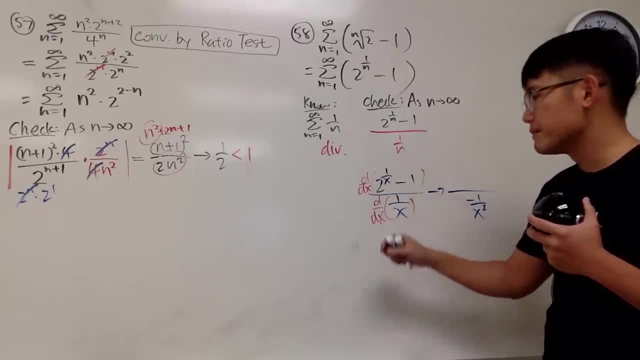 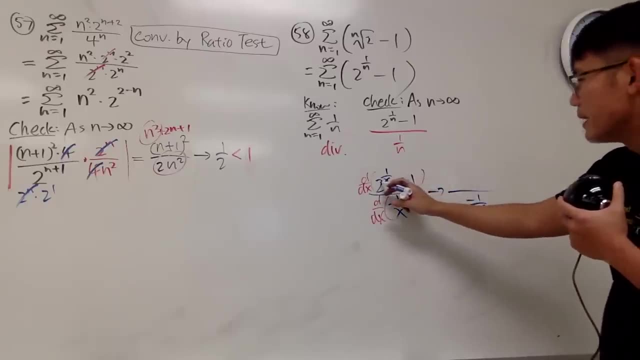 right here. when we have b to the exponential function, let's say sorry. when we have b to a power, and for the function, it's a. if the power is a function, we just first maintain this, which is 2 to the 1 over x power. but 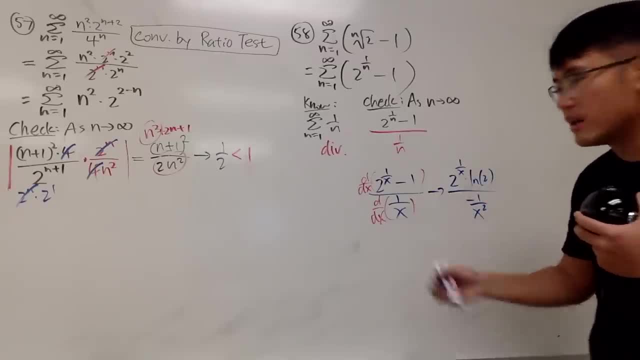 you have to multiply by natural log of 2 because of the base, is not e? right? if you have e to the whatever, it's just e to the whatever, times, l and e, that kind of thing. so that's the idea. however, you still have to multiply by. 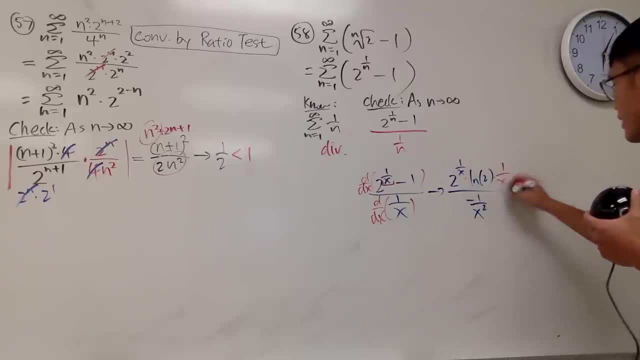 the derivative of 1 over x, which is- I don't think we are doing the luchen today, unfortunately, but anyway, cancel, cancel. when x goes to infinity, this is 0. this is just going to be 1. in another word, this right here gives us ln 2. 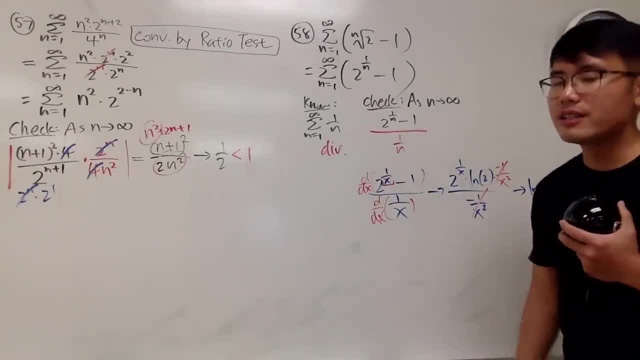 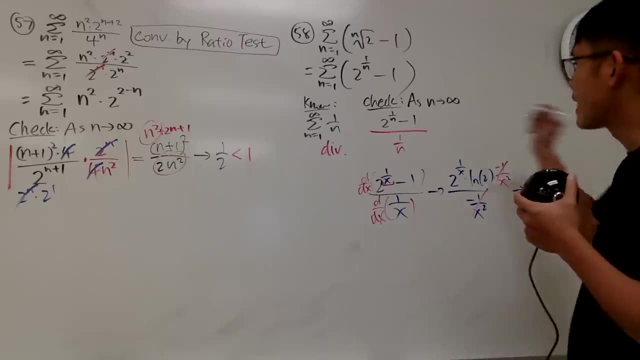 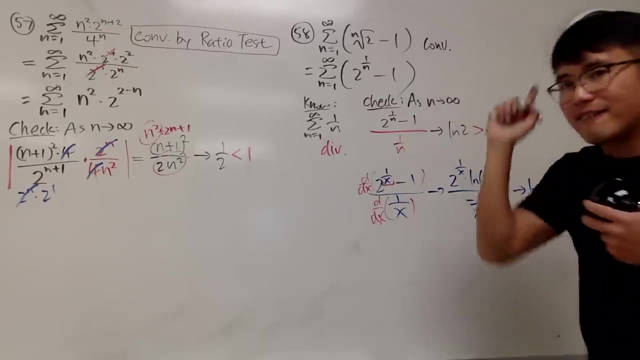 very nice, isn't it? we are doing the limit comparison test, so this right here is useful because it's greater than 0, so we can come back here and first say: this right here is 0, this right here converges: no, actually no, what's my mistake? 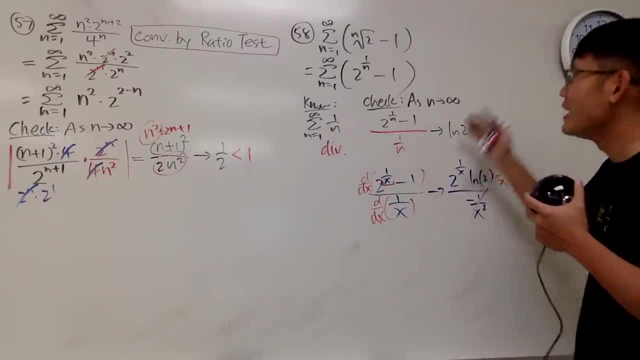 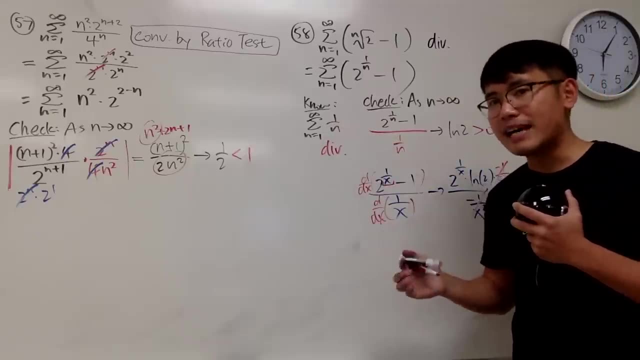 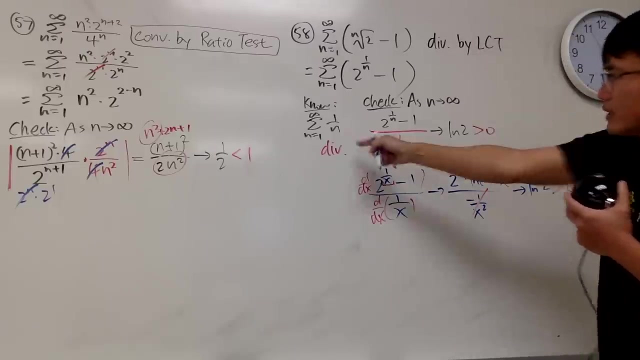 because we are using the divergent. they have to have the same conclusion, right? so this right here diverges. this and that are pretty much have the same size. this right here diverges because the limit comparison test with that guy, right? take a look, take a look. 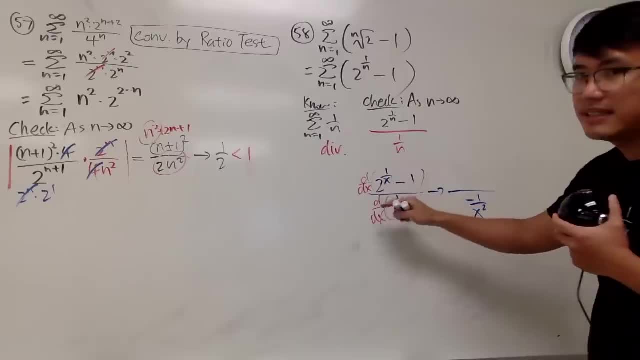 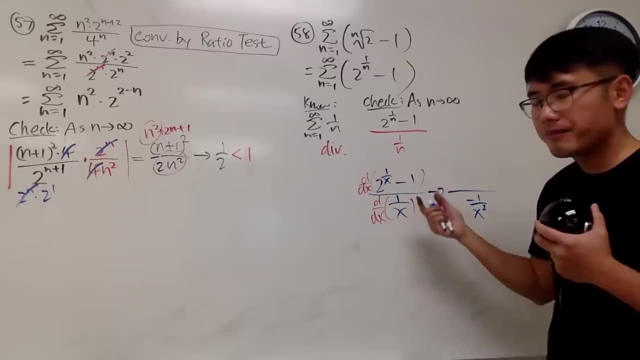 That's nice. The derivative of this is just gone, Nice, Right here. when we have b to the exponential function, sorry, when we have b to the power and the function is, if the power is a function, we just first maintain this. 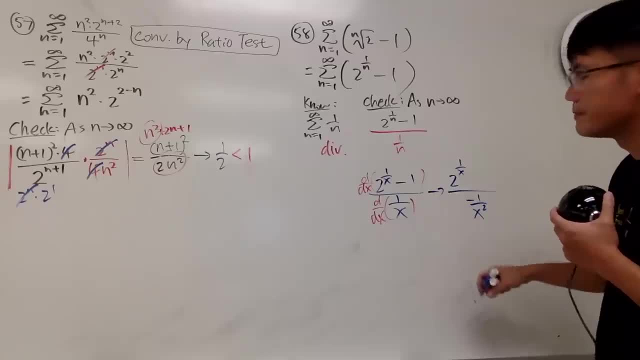 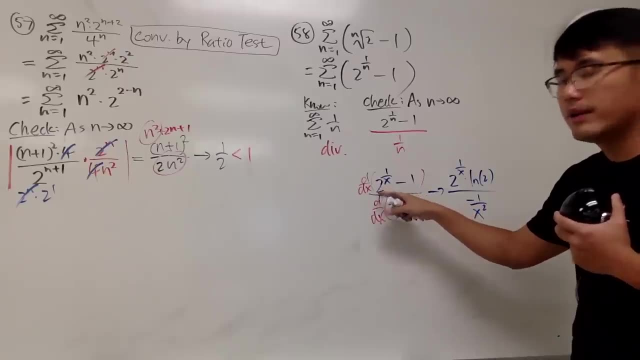 which is 2 to the 1 over x power. But you have to multiply by natural log of 2.. Because of the base, is not e Right? If you have e to the whatever, it's just e to the whatever. 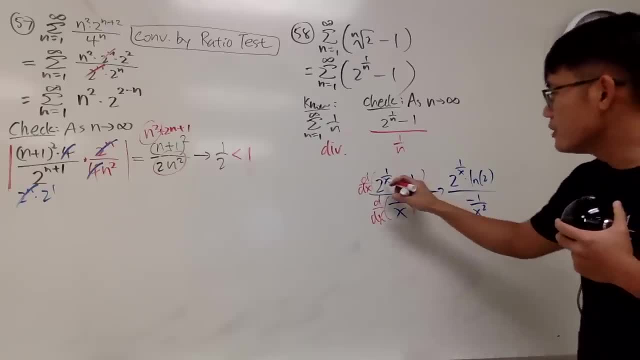 times l and e, that kind of thing. So that's the idea. However, you still have to multiply by the derivative of 1 over x, which is the chain loop right. I don't think we are doing the loop chain today. 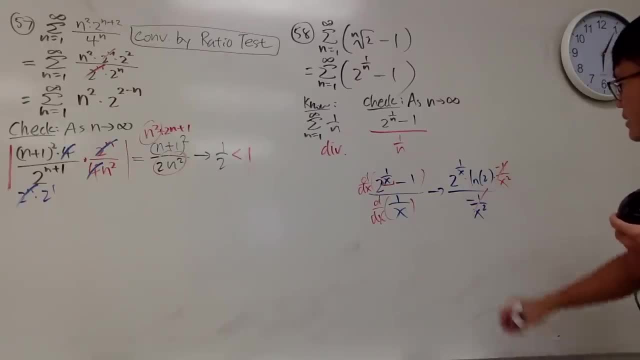 unfortunately, But anyway, cancel, cancel. When x goes to infinity, this is 0,, this is just going to be 1, in another word, this right here gives us ln 2.. Very nice, isn't it? 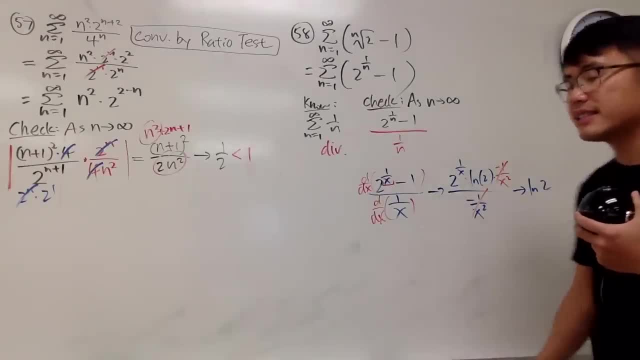 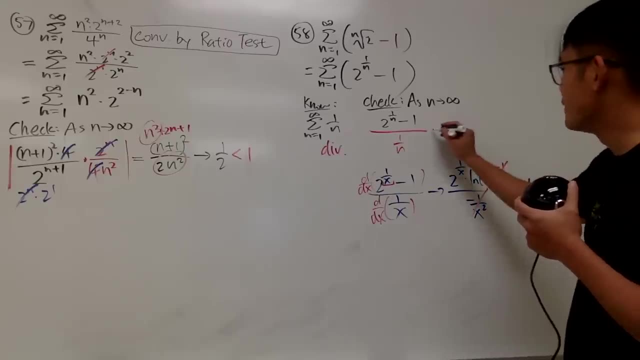 We are doing the limit comparison test. So this right here is useful because it's greater than 0.. So we can come back here and first say this right here is approaching ln 2, which is greater than 0. This right here 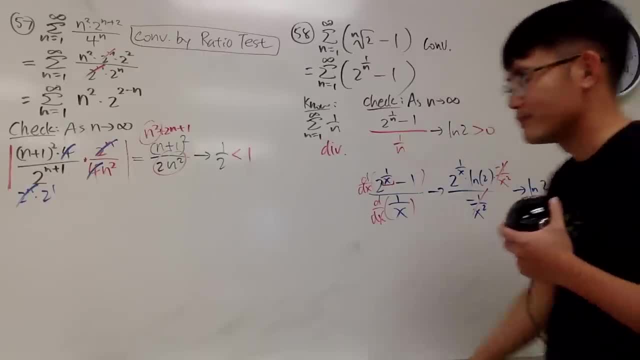 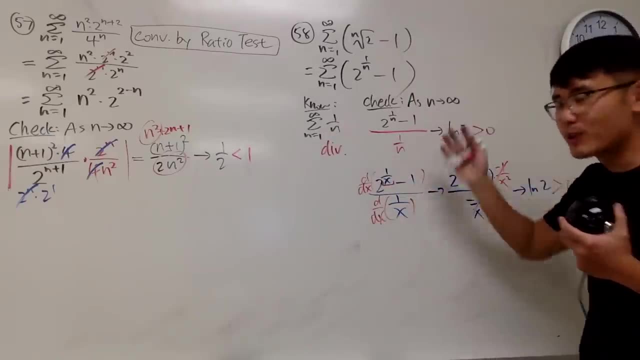 converges. no, actually no, What's my mistake? Because we are using the divergence. they have to have the same conclusion, right. So this right here diverges. This and that are pretty much of have the same size. 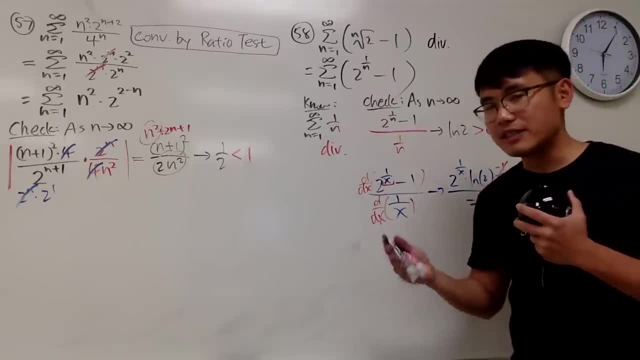 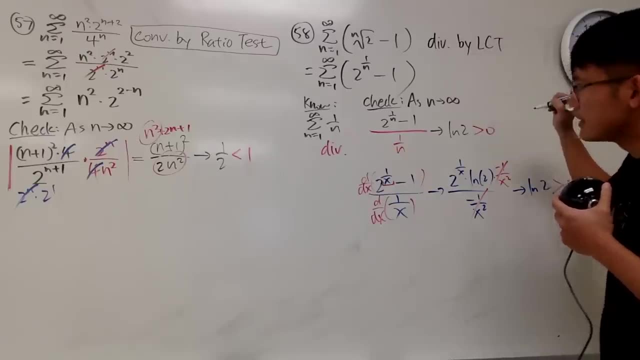 This right here diverges because the limit comparison test with that guy, right. So take a look, take a look, take a look like that, Okay, So this right here diverges because the limit comparison test. 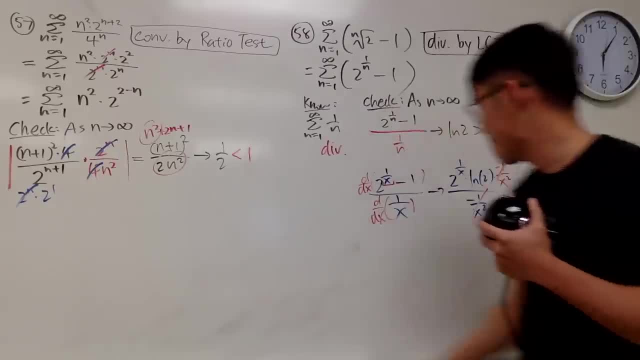 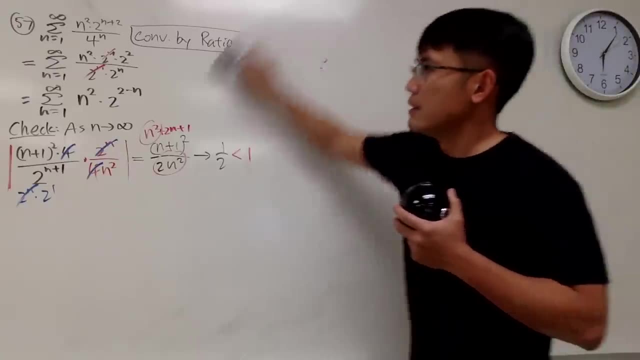 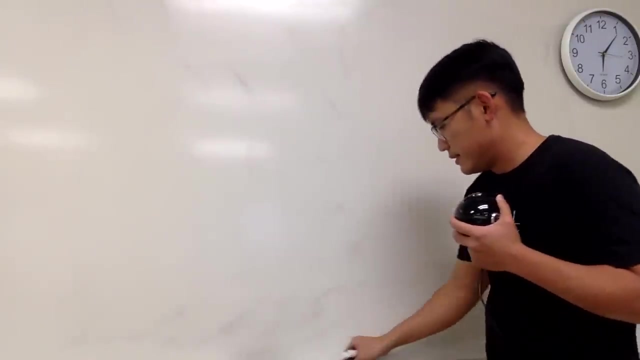 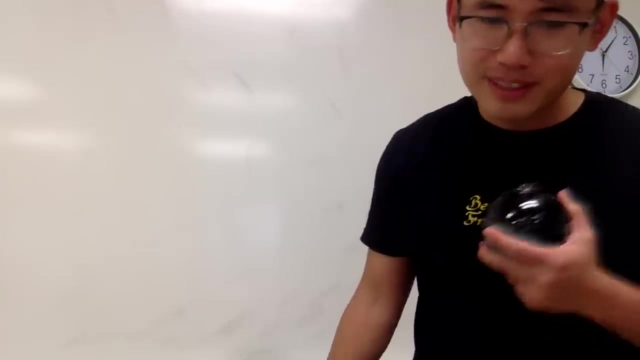 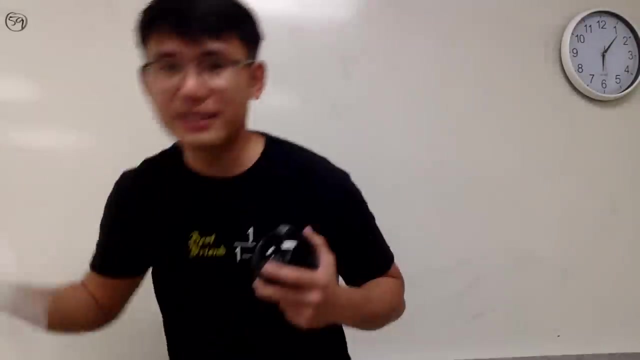 with that guy, right? So take a look, take a look like that. Well, the next one is trickier. That's the number 59, right here, These are the ones that I finished. Now those questions. 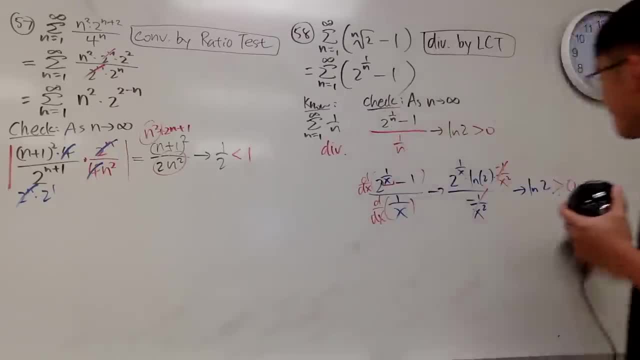 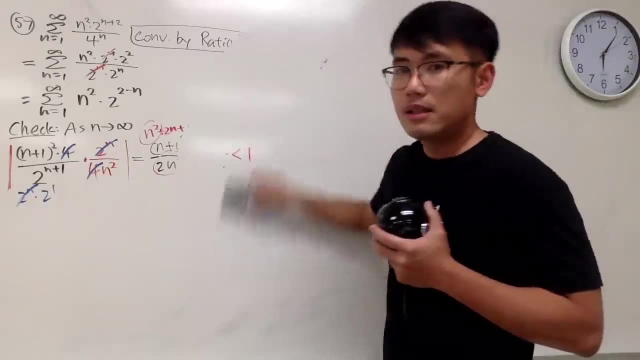 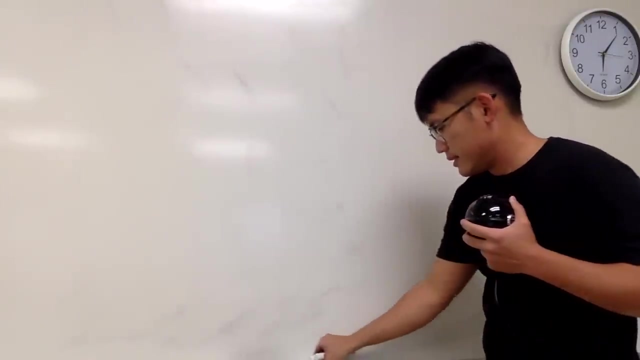 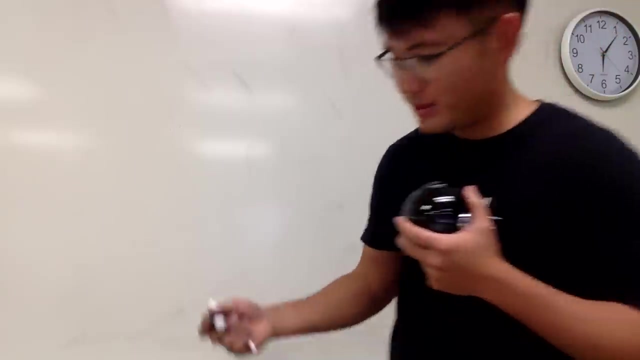 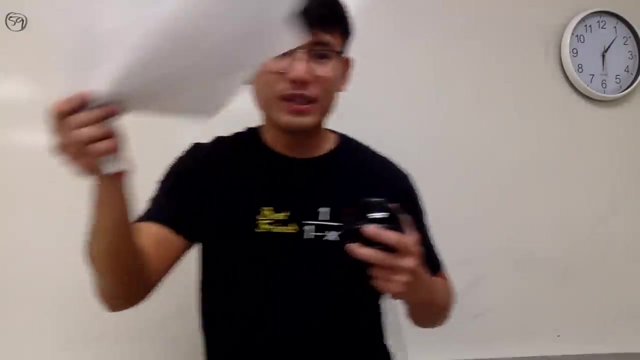 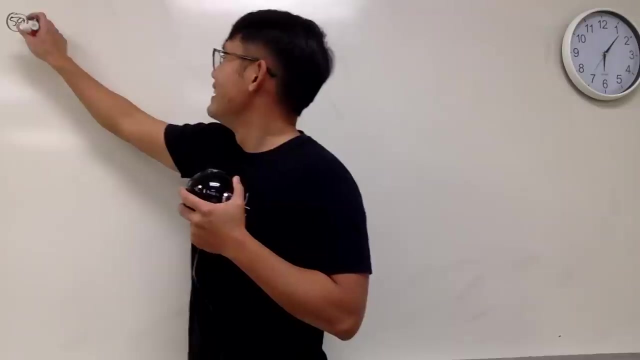 like that. okay, well, the next one is trickier. let's see number 59. these are the ones that I finished. now two questions. number 59: we have the sum as n goes from 1 to infinity, the nth root of 2 minus 1, and. 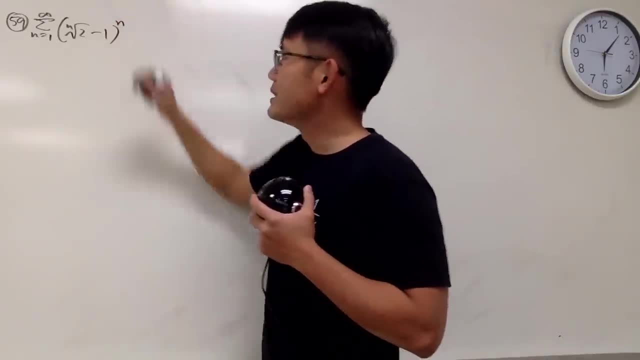 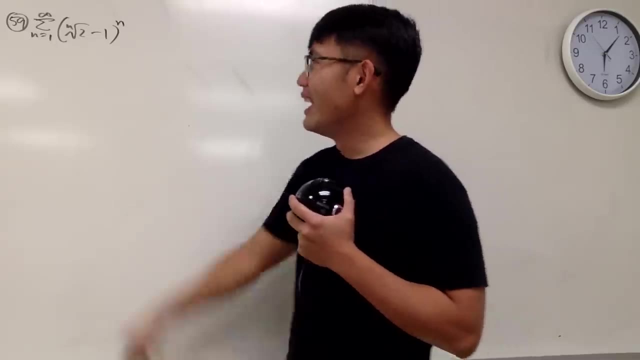 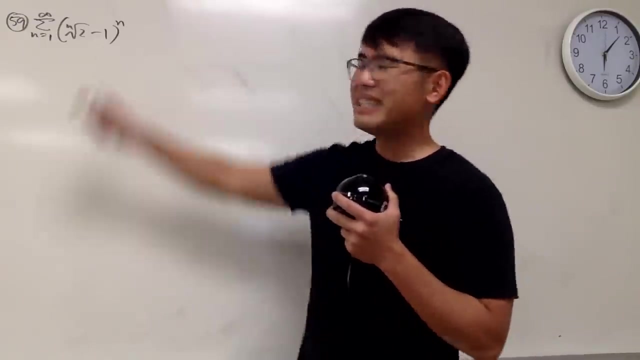 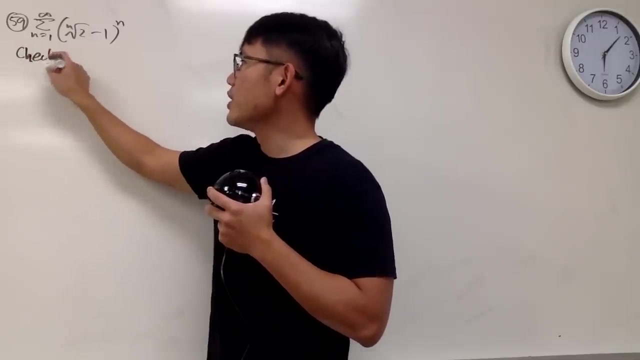 we take this to the nth power. okay, so, unlike earlier. okay, so you can try however you want, but this is what we want to do. I see the n in the exponent, so let me use the root test. right, so I will try to use the root test. 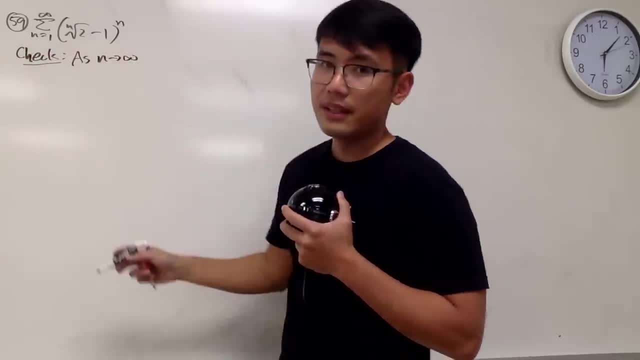 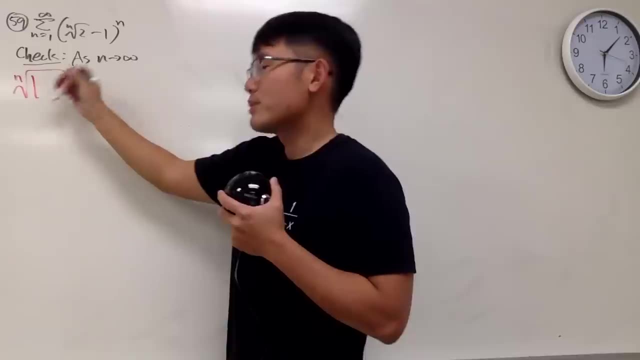 and this is the things that we are going to check. if we are using the root test, as n goes to infinity by the root test, first we take the nth root with absolute value, but we don't need to, but this right here is the same as n. 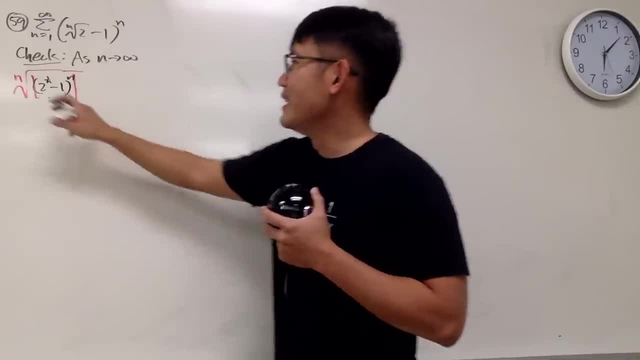 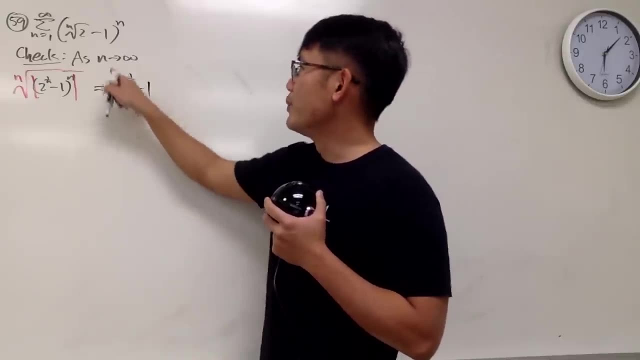 2 to the 1 over. nth power, absolute value doesn't matter in this case. n and n cancel out, so we just end up with 2 to the 1 over, n minus 1, and if you put infinity in here, you get 2 to the 1 over. 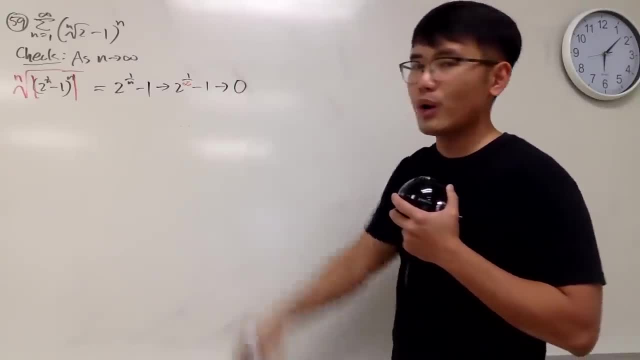 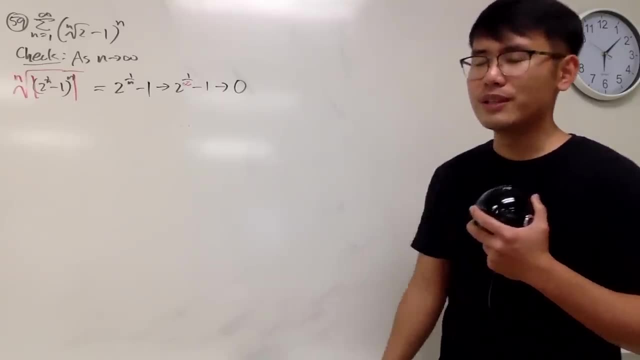 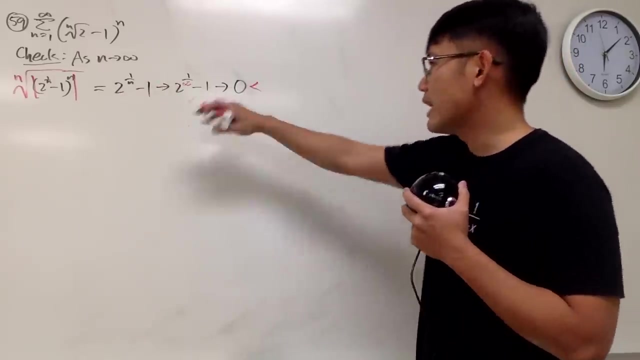 infinity minus 1, which is approaching 1 minus 1, which is 0. this right here is the root test. so does 0 do us any good? yes, root test says: if the result is 0 for that limit, if this is less than 1. 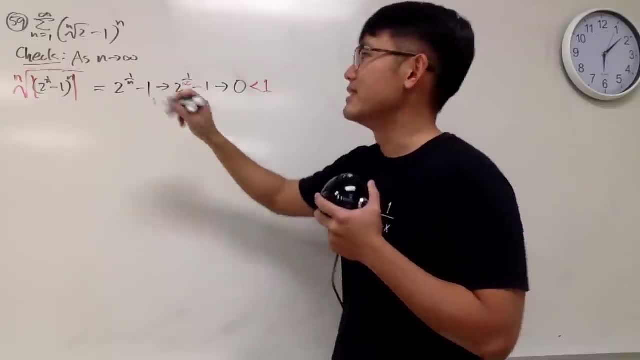 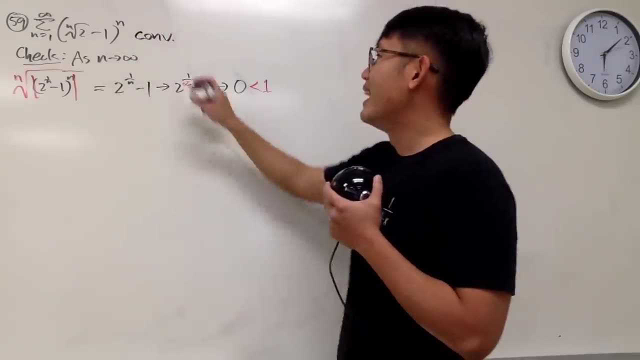 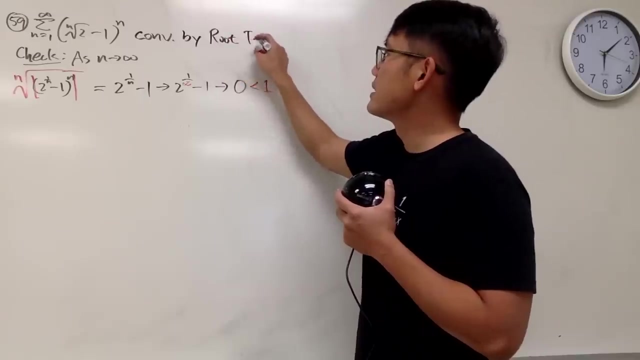 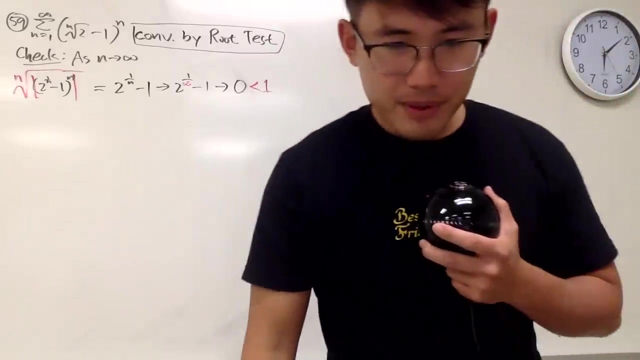 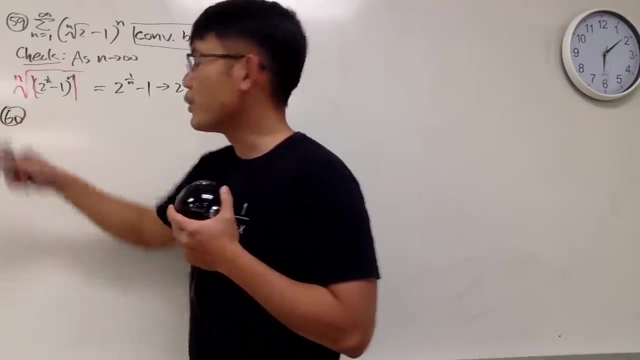 which is 0 is less than 1. we can come back here and draw our conclusion and say this: right here, actually converges, converges, converges, converges by the root test, right? so just like that, now we have a very simple formula for the sequence. 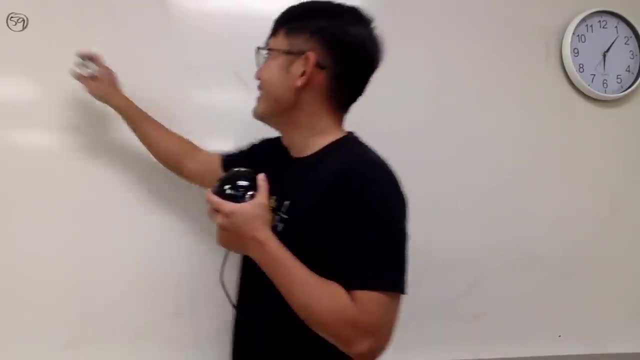 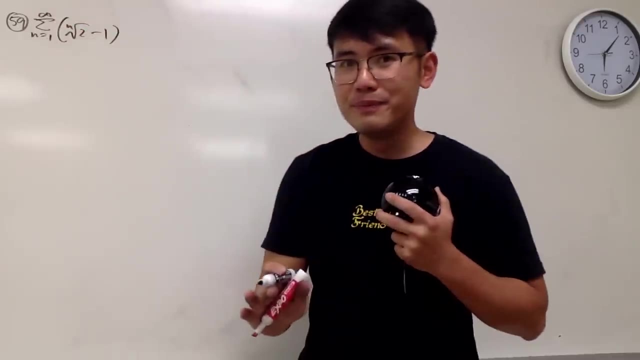 Number 59, we have the sum, as n goes from 1 to infinity, the nth root of 2 minus 1, and we take this to the nth power. Yeah, Okay, So unlike earlier, you. 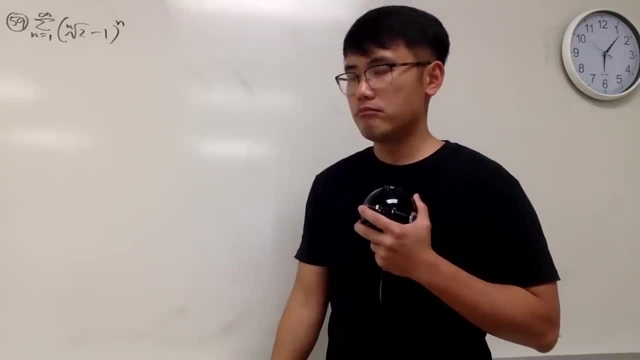 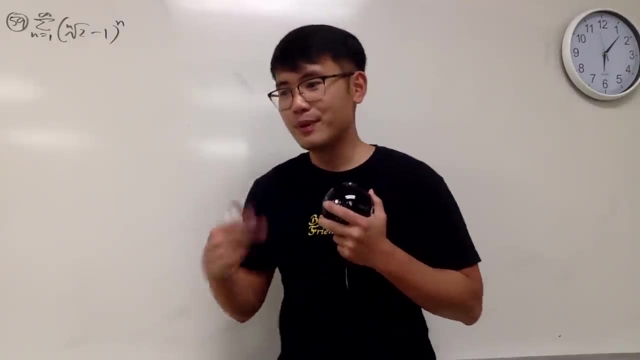 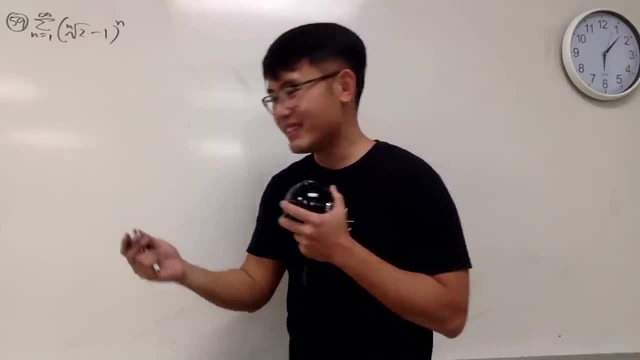 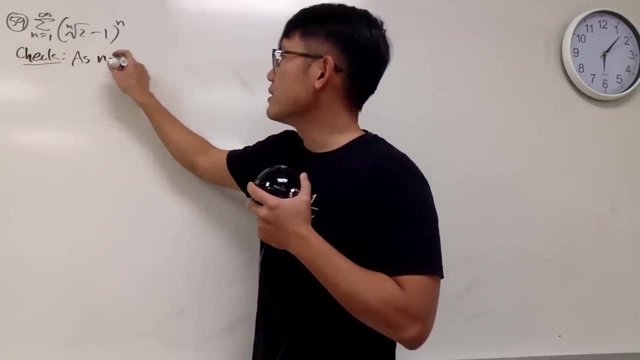 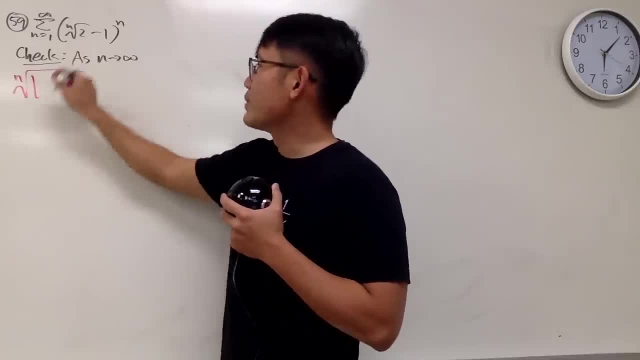 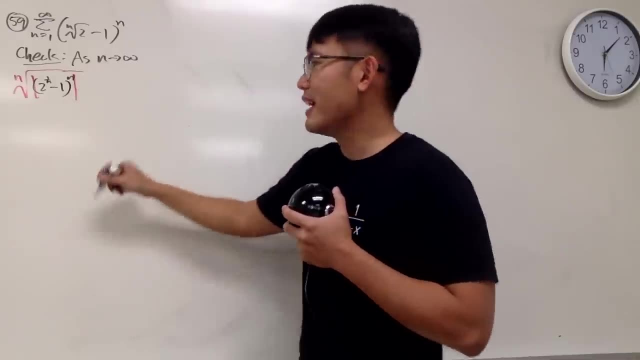 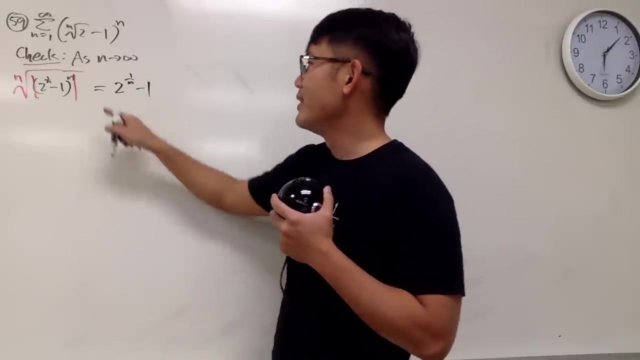 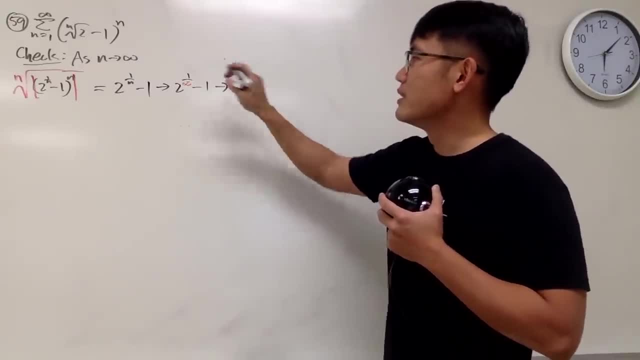 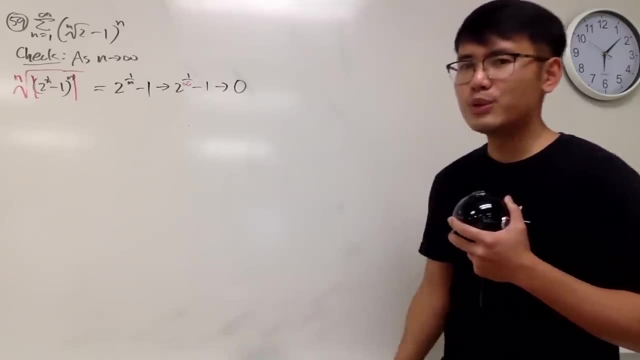 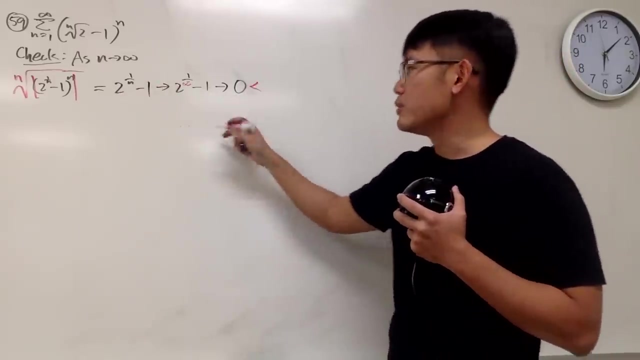 which is approaching 1 minus 1, which is 0. This, right here, is the root test. So does 0 do us any good? Yes, Root test says if, when you are doing this right here, if the result is 0 for that limit. 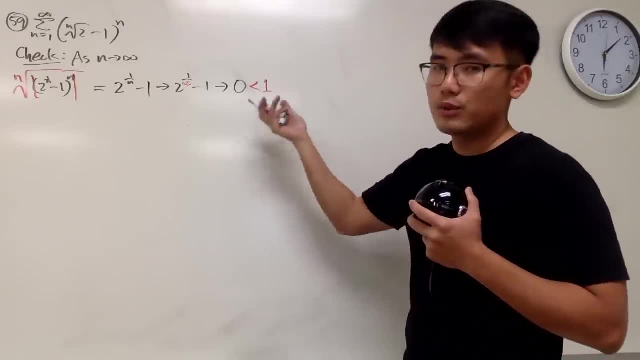 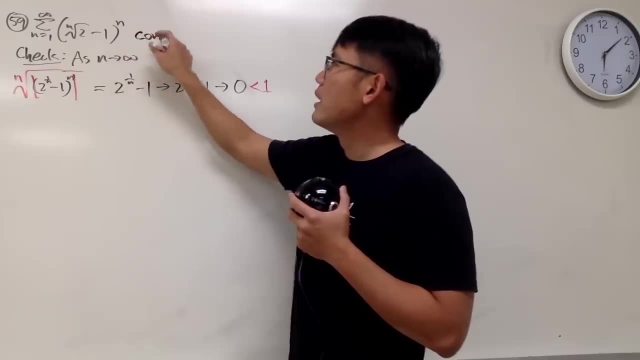 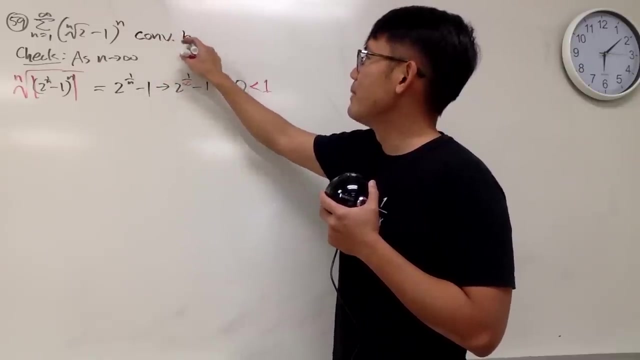 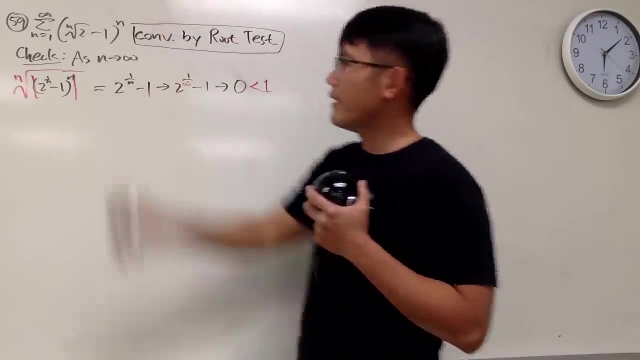 if this is less than 1, which is 0 is less than 1, we can come back here and draw our conclusion and say this: right, here, actually converges, converges, converges, converges by the root test, right, so just like that. Now number 61: 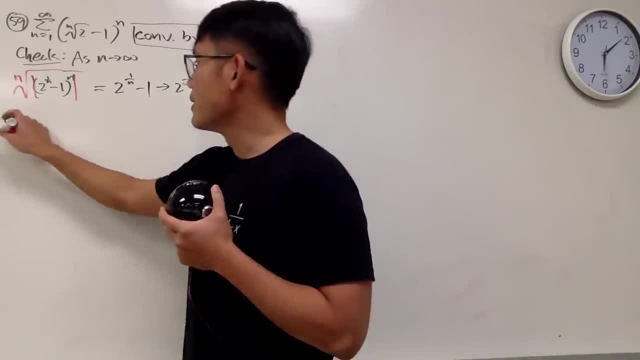 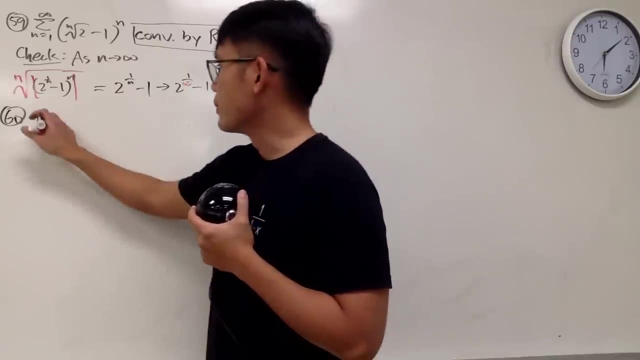 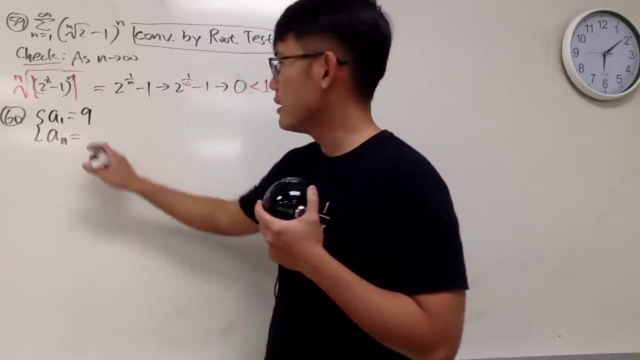 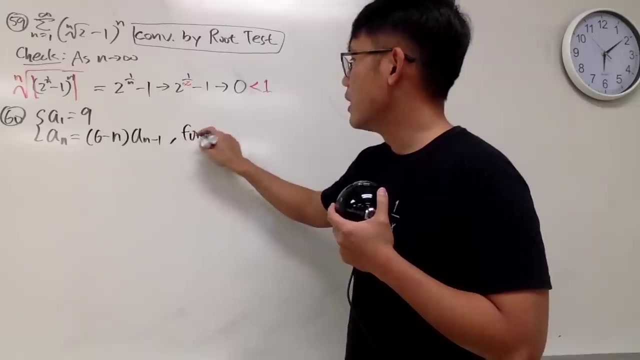 this time I'm going to give you guys a recursive formula for the sequence and then we'll find out the sum for that. So I'll just tell you, given a1 is equal to 9, an is equal to 6 minus n times the previous term, namely an minus 1, and this is true for n is greater than or equal to 2, like. 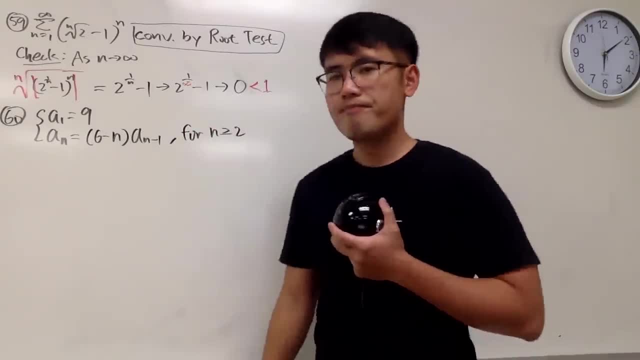 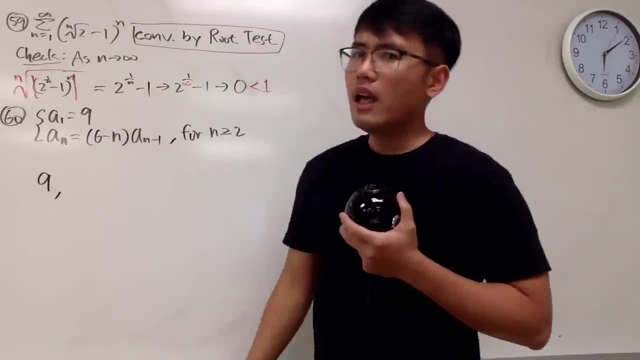 this. Let's don't worry. let's just write down a few terms to see what happens. First of all, a1 is 9.. a2 is what? Well, remember this is going to be n equal to 2, so you have to use this formula to get. 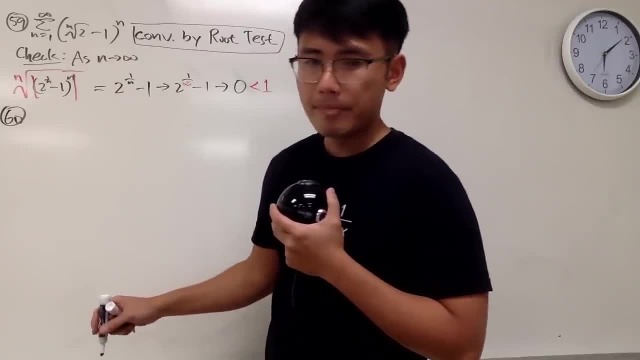 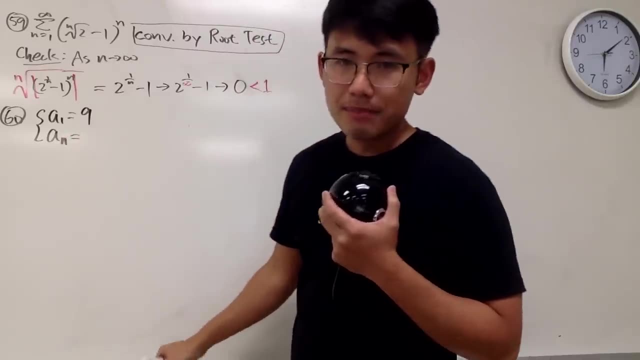 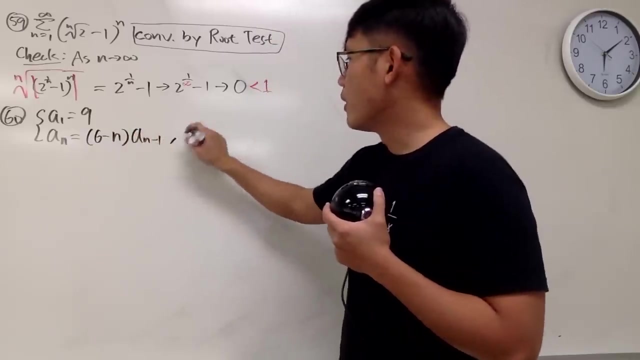 and then we'll find out the sum for that. so, hmm, I'll just tell you, given a1 is equal to 9, an is equal to 6 minus n times the previous term, namely an minus 1, and this is true for n is greater than. 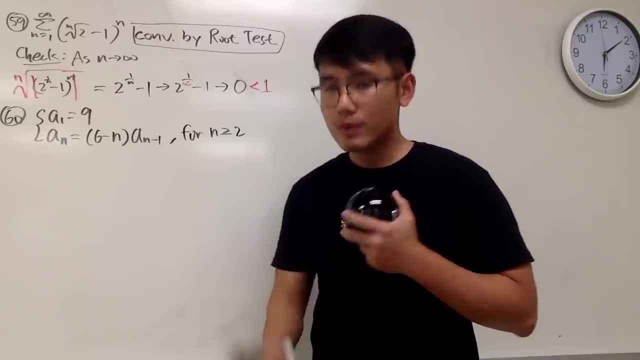 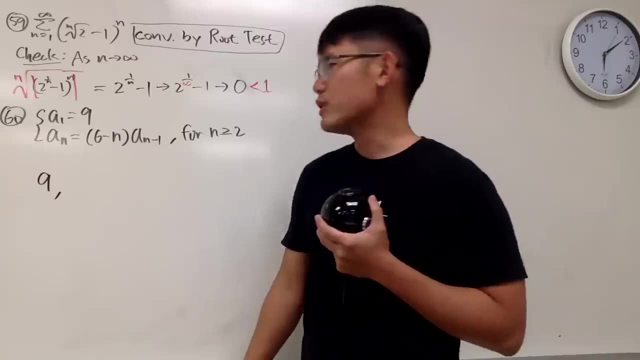 or equal to 2. let's don't worry. let's just write down a few terms to see what happens. first of all, a1 is 9, a2 is what well remember. this is going to be n equal to 2, so you have to use: 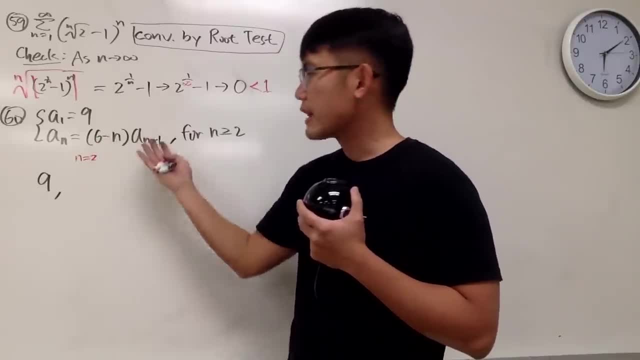 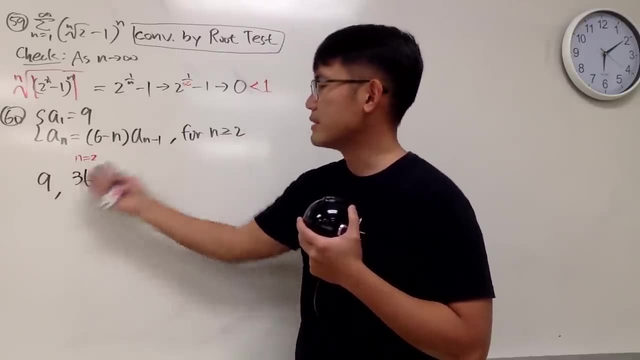 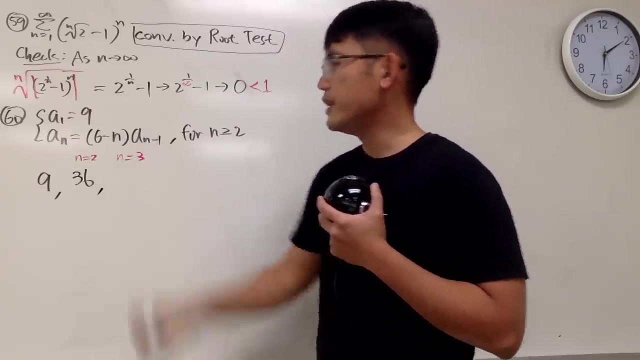 this formula: to get a2, first of all you do 6 minus 2, which is 4 times the previous term, which is 36, like that. okay, so again is 4 times 9. let's do the next one. let's see: n equals 3. 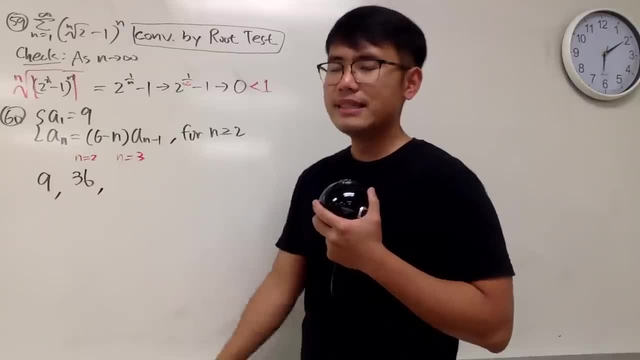 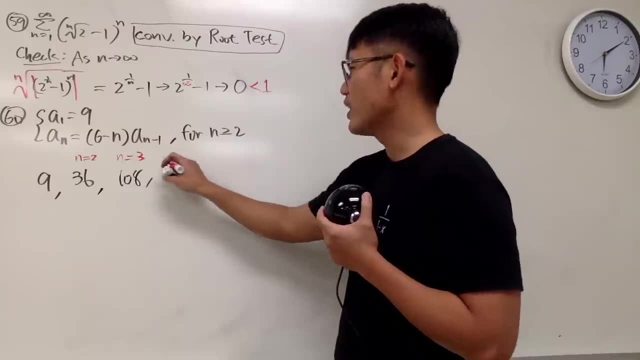 that's going to be 3 and you multiply by the previous term. 3 times 36 is 108. oh my god, it's getting bigger and bigger. okay, n equals 4. put 4 in here. this is going to give you 2 times the previous term. 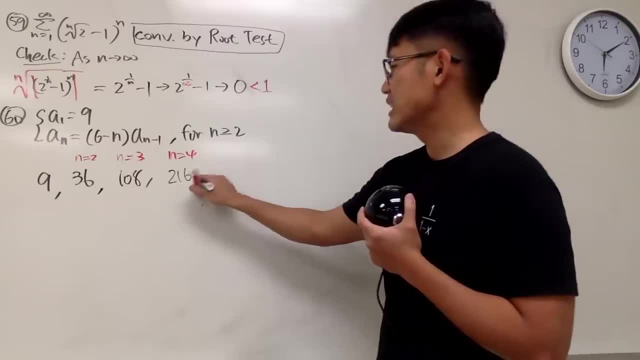 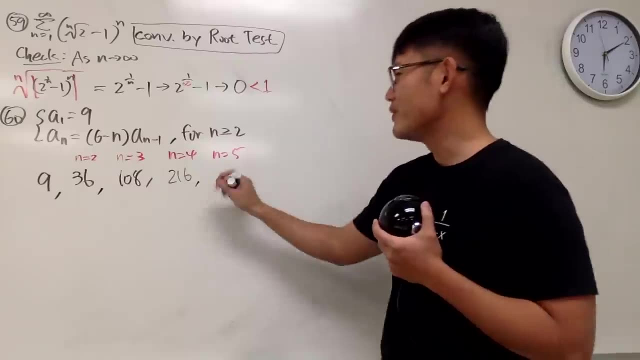 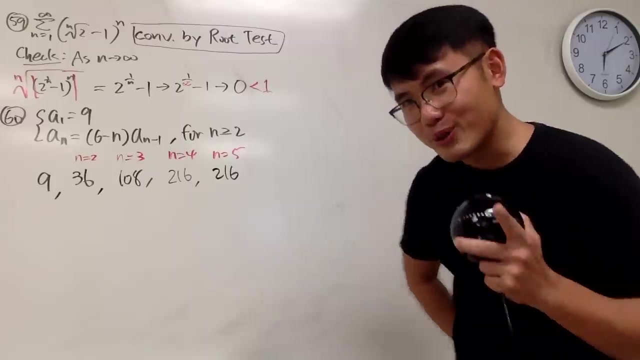 we get 216. ah n equals 5. am I really doing this right? 1 minus a? 6 minus 5 is 1, 1 times the previous one is 216. okay, I want to give up, but no, don't give up, because the next one. 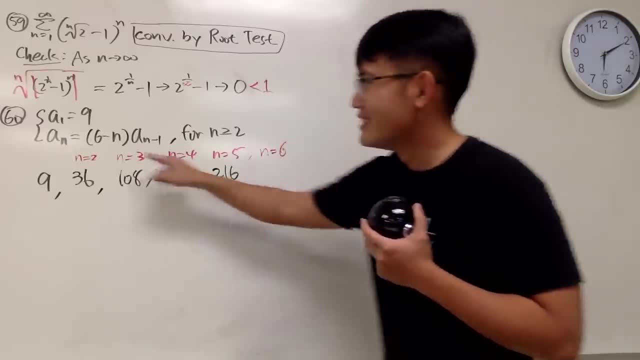 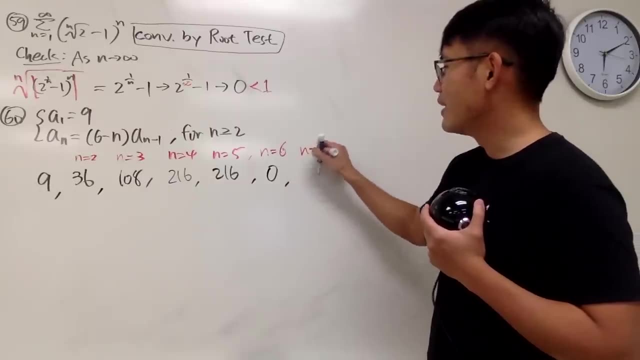 n equal to 6, what happens? we will get 6. in fact, 6 minus 6 is 0, 0 times this guy is 0. what's the next guy? n equal to 7. well, you get negative 1 times the previous term. 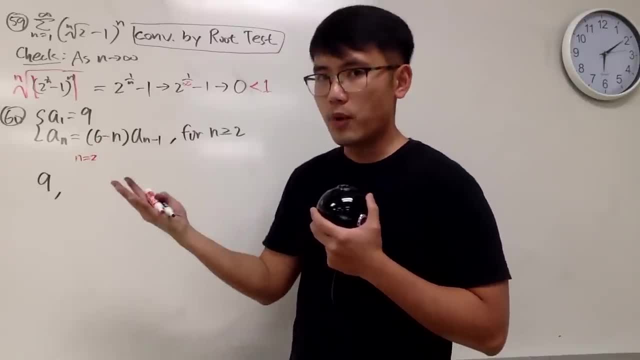 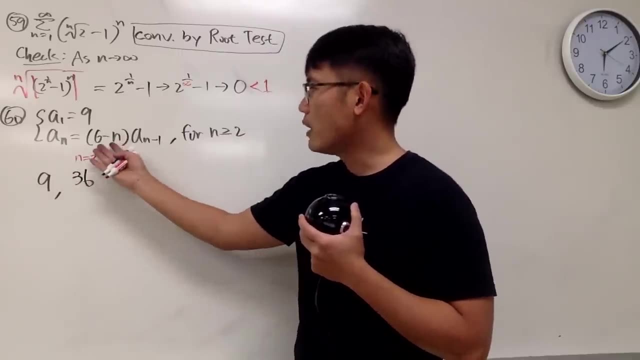 a2.. First of all, you do 6 minus 2, which is 4 times the previous term, which is 36, like that. okay, so again is 4 times 9, 4 times the previous term, like that. and we do the next one, that's the n equals. 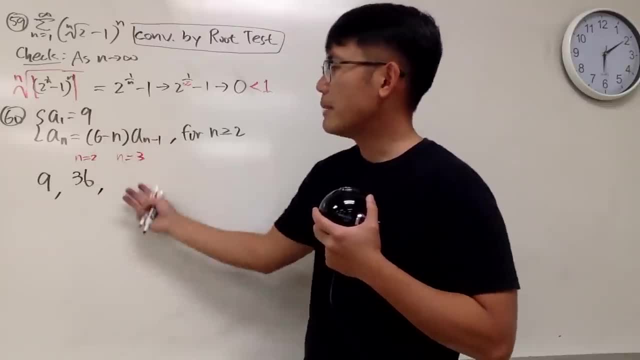 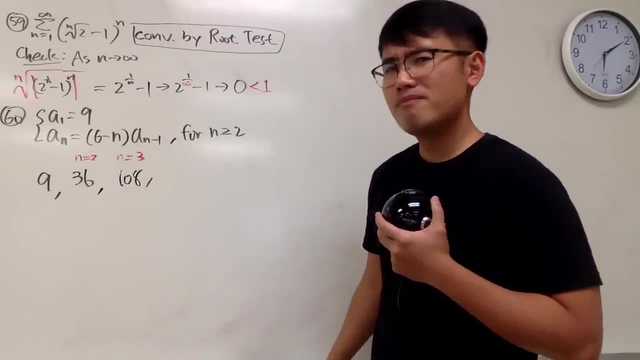 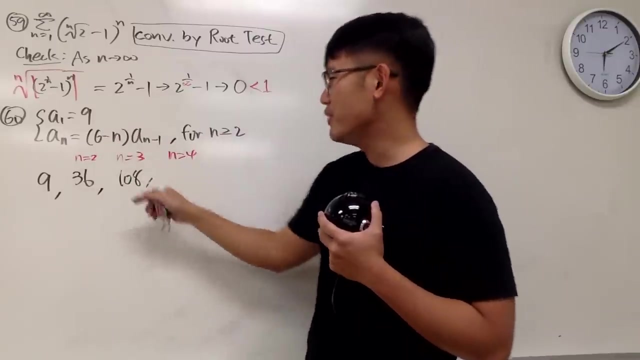 3, that's going to be 3, and you multiply by the previous term. 3 times 36 is 108. oh my God, it's getting bigger and bigger. okay, n equals 4, put 4 in here. this is going to give you 2 times the previous term. we get 216. 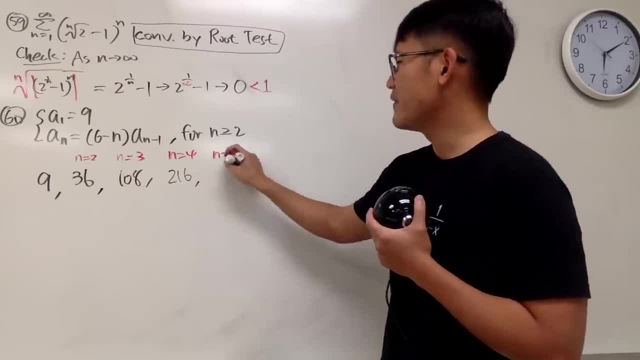 Ah, n equals 5. am I really doing this right? 6 minus 5 is 1: 1 times the previous, 1 is 3.. is 1: 1 times the previous one is 6.. 1 times the previous one is 6.. 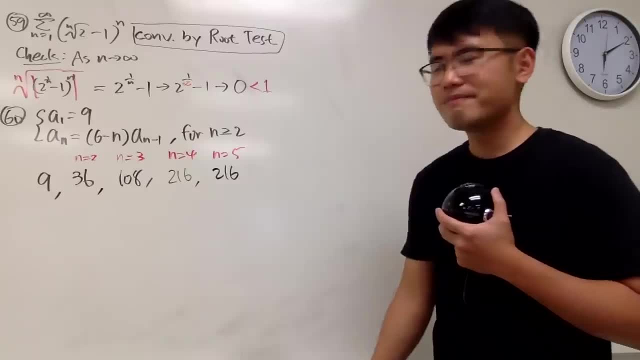 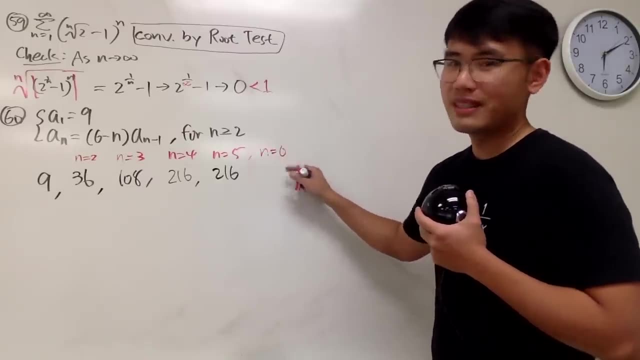 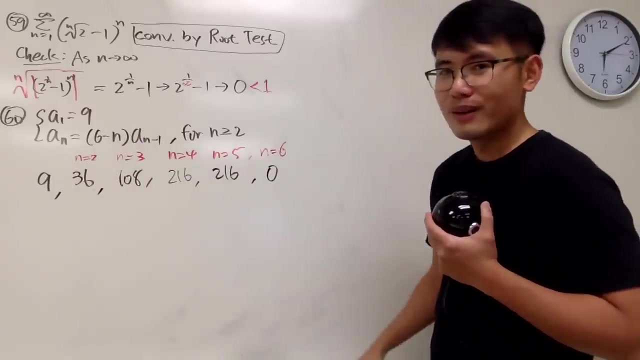 1 times the previous one is 6.. is 216.. Okay, I want to give up, But no, don't give up, Because the next one n equal to 6, what happens? We will get 6.. 6 minus 6 is 0.. 0 times this guy is 0.. What's the next? 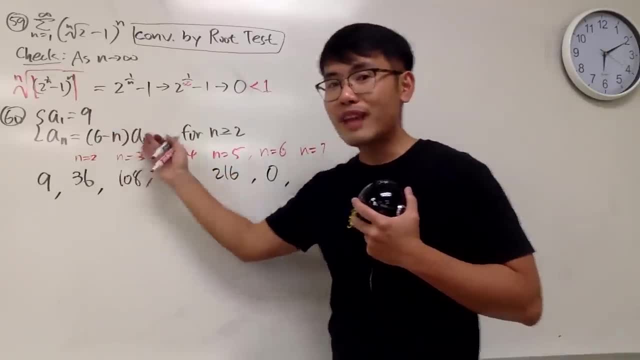 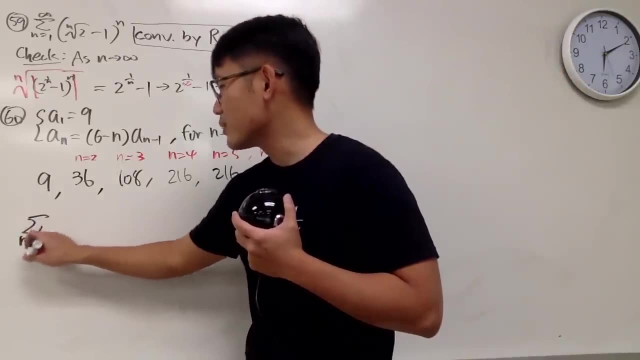 guy n equal to 7.. Well, you get negative 1 times the previous term, which is 0.. Da-da-da-da-da-da-da. So in this question here, if you want to find out the sum as n goes from 1 to infinity. 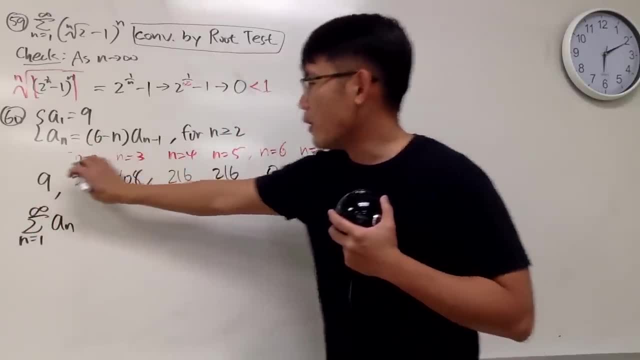 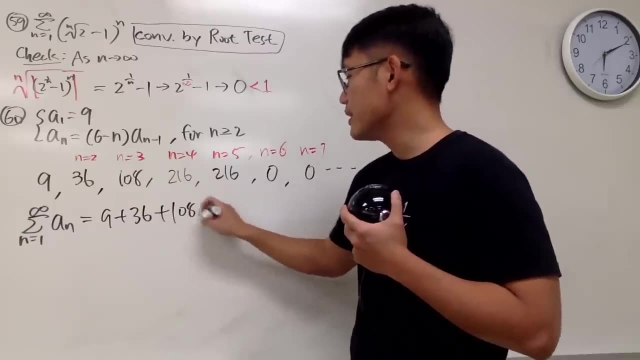 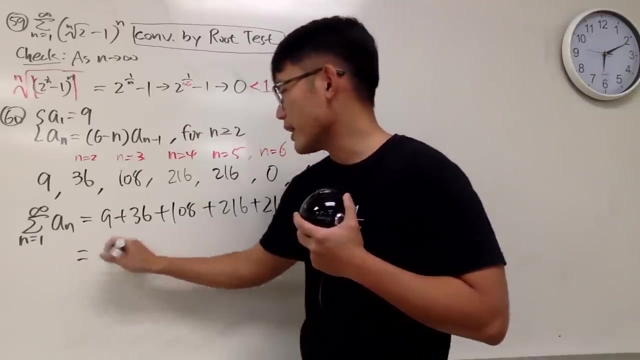 of this, the sum of all this. right here, all we have to do is just 9 plus 36, plus 108 plus 216 plus 216, like this, And I want you guys to help me. okay, I want you guys to comment. 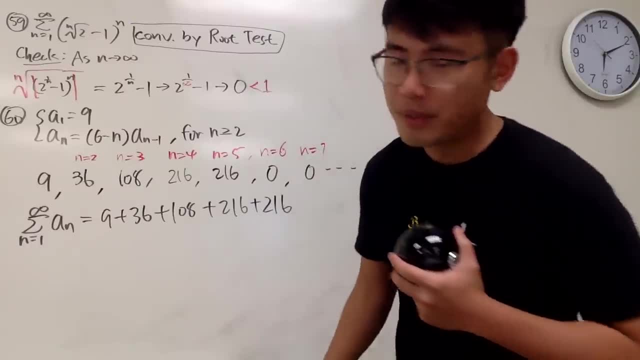 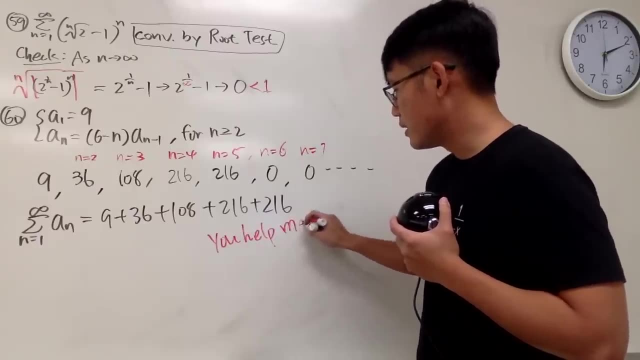 down below the answer because it's been so many hours so you are going to need to help me because, seriously, you back me up for this one. you help me right. and of course, on the test, you cannot just put on your. help me on the test, you really. 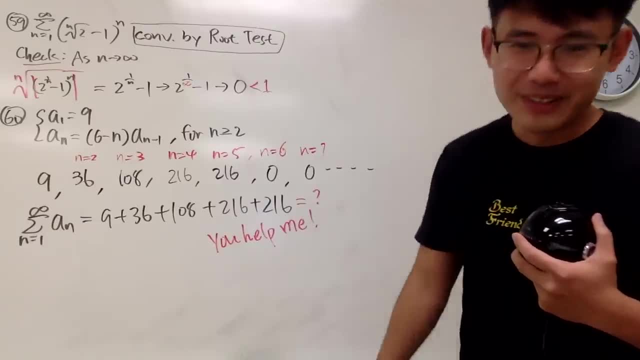 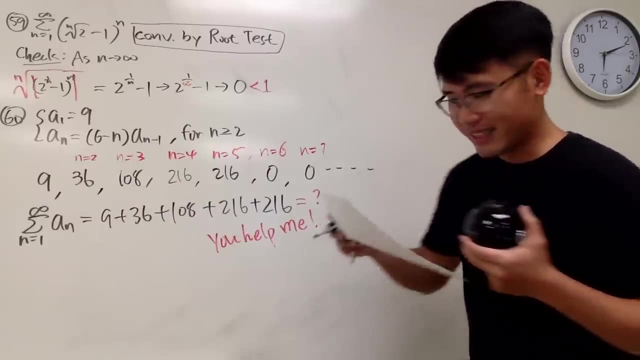 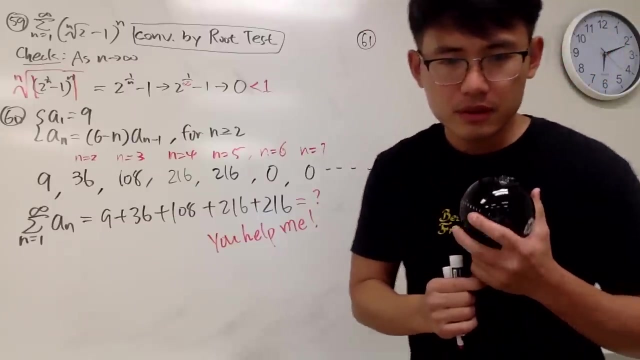 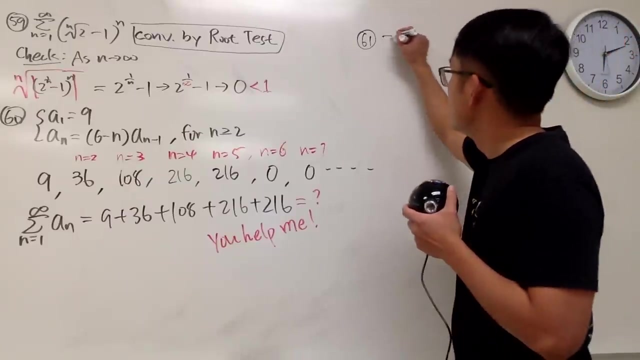 have to use the calculator to do the work and tell me what the answer is. okay, so don't be like me on the test. that's no good, that's bad as dangerous. okay, number 61, right here. okay, the sum as n goes from 1 to infinity, and. 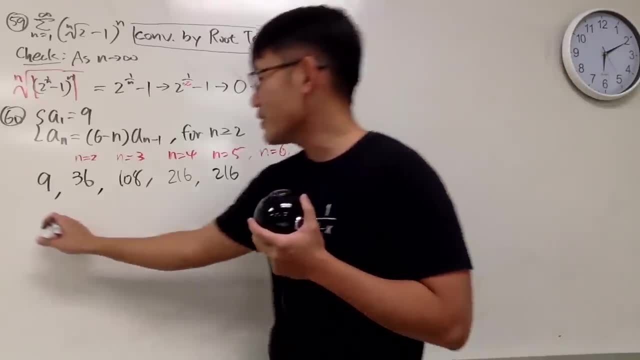 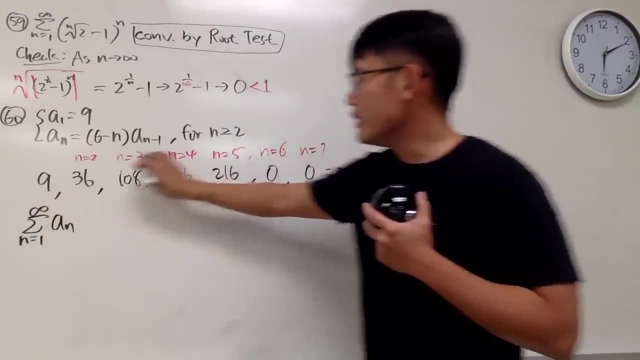 which is 0, da, da, da, da, da, da da. so this question here: if you want to find out the sum, as n goes from 1 to infinity, of this, um, the sum of all this, right here, all we have to do is just 9 plus. 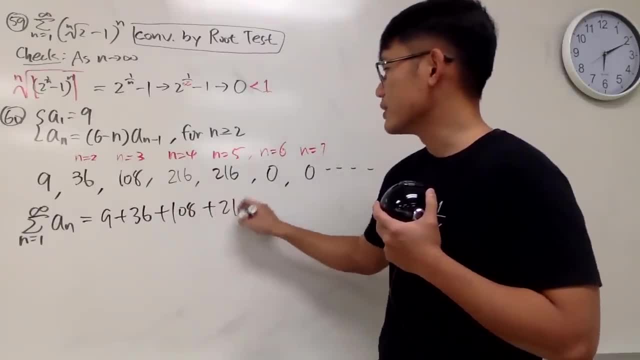 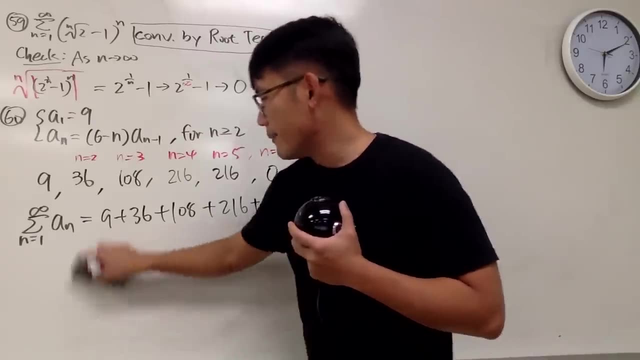 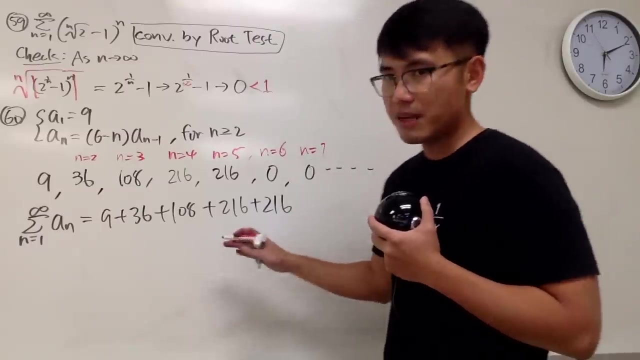 36 plus 108 plus 216 plus 216, like this, and I want you guys to help me. okay, alright, I want you guys to comment down below the answer because, ah, it's been so many hours so you have got to help me. okay, you back me up? 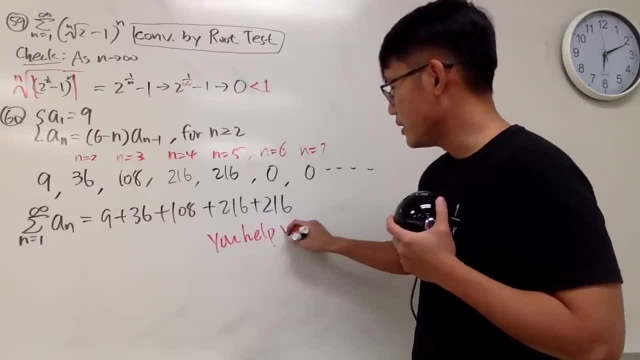 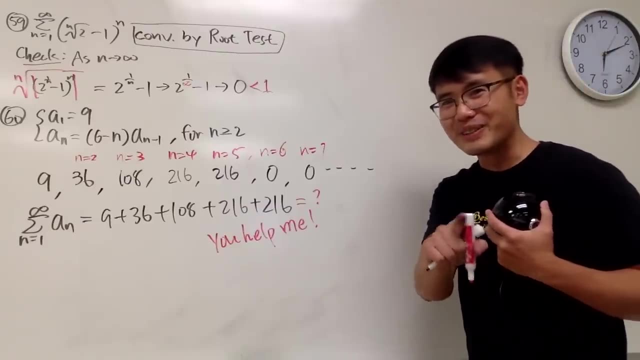 for this one, you help me right and, of course, on the test, you cannot just put on. you help me on the test. you really have to use the calculator to do the work and tell me what the answer is. okay, so don't be like me on the test. 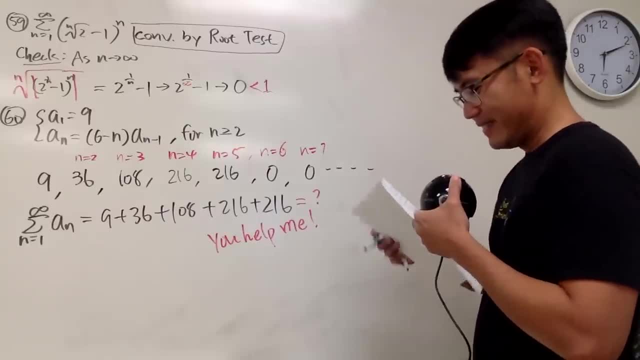 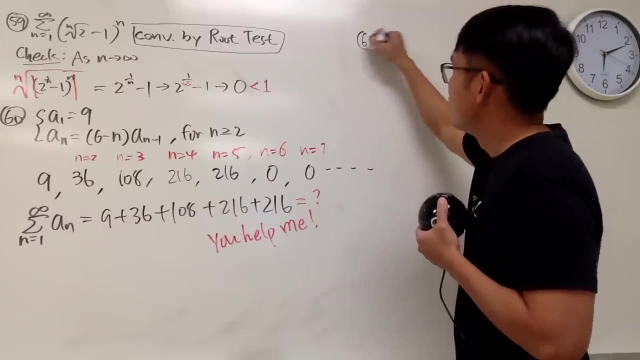 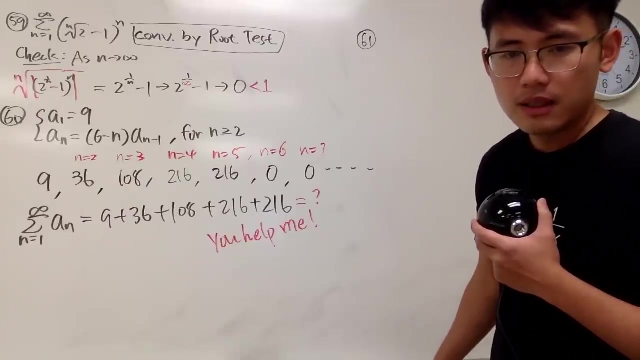 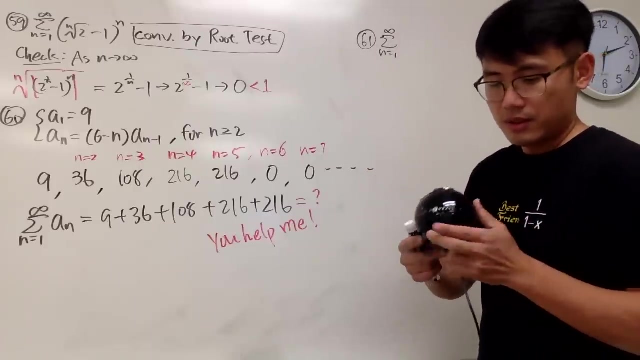 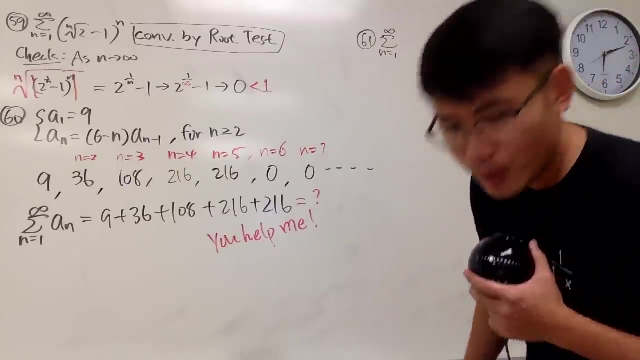 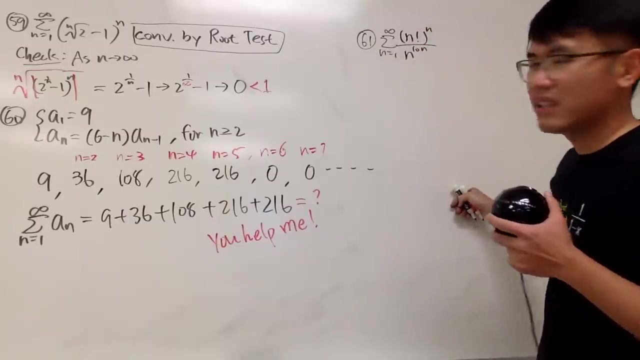 that's no good, that's bad, that's dangerous. okay, number ah 61 right here. okay, let's see the sum as n goes from 1 to infinity and n factorial to the nth power, n factorial to the nth power, over n to the 10 nth power. 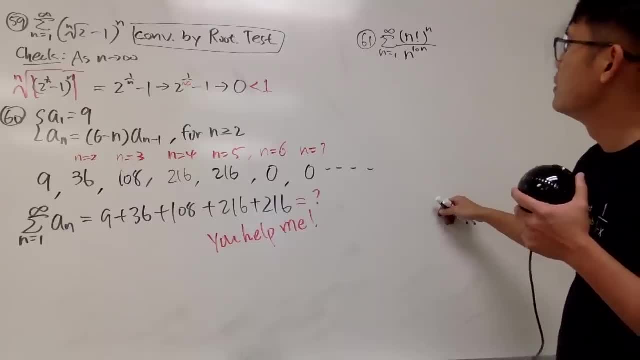 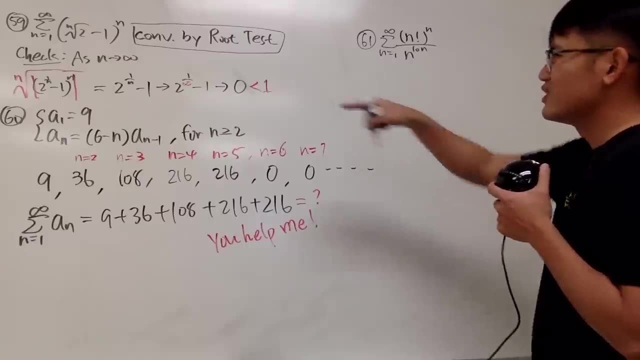 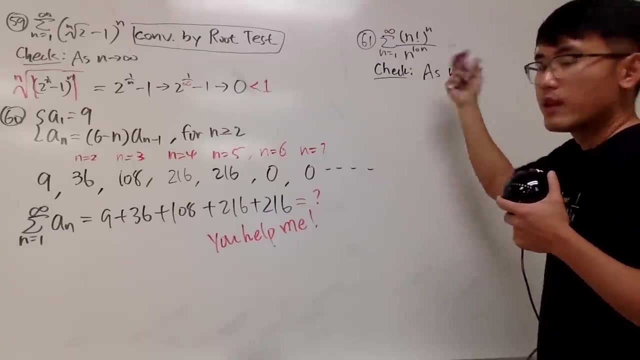 god, whoa. Well, we have the power that has n, so let's do the root test. It's just like that. So here we go, Let's go check, As n goes to infinity. here I'm just going to take the nth root: absolute value. 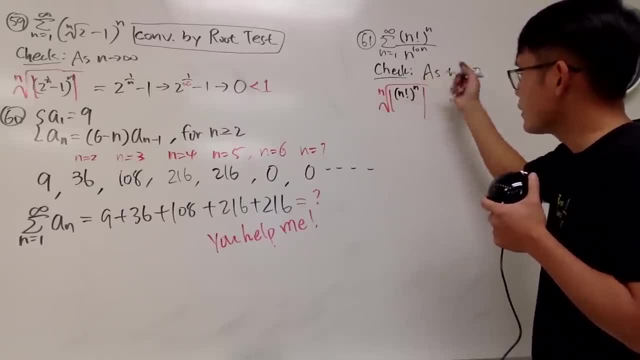 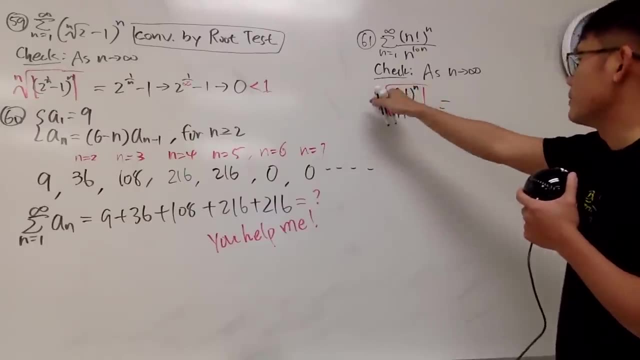 and here we have n factorial and you raise that to the nth power, which is like humongous. Anyway, n and n will be gone because you are dividing it because of the nth root, and then the absolute value doesn't make, doesn't, doesn't, doesn't do anything anymore. 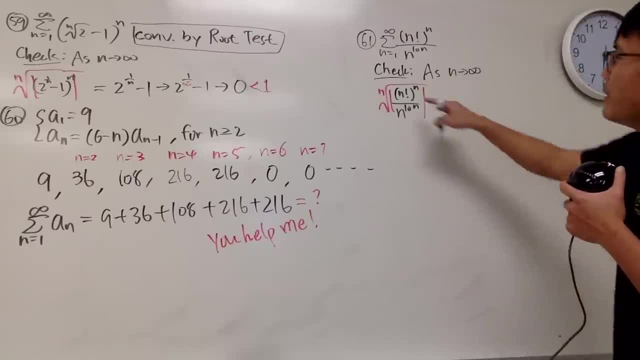 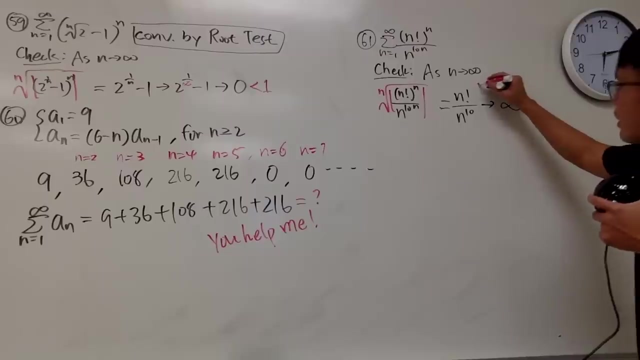 It doesn't, really doesn't matter. Anyway, here we have n factorial over n to the nth power. So what's the conclusion for this guy? It goes to infinity, because this right here is so much bigger than the bottom one. Why, How do we know? 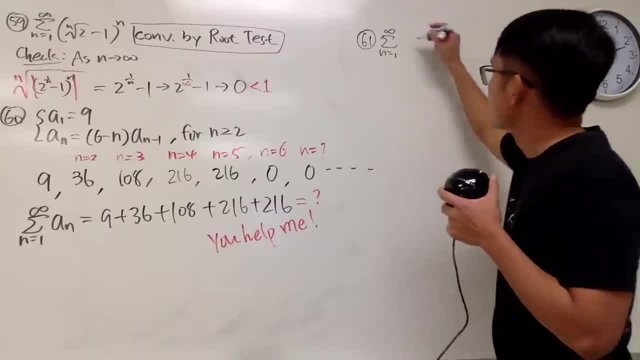 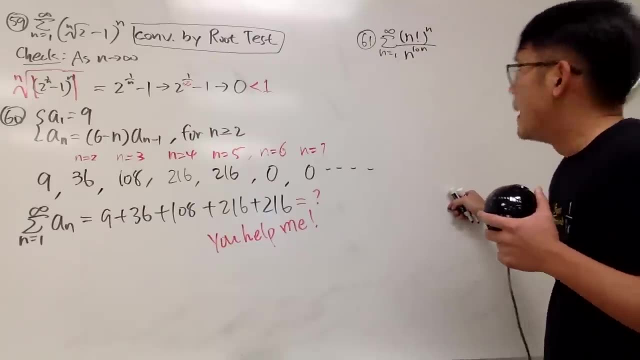 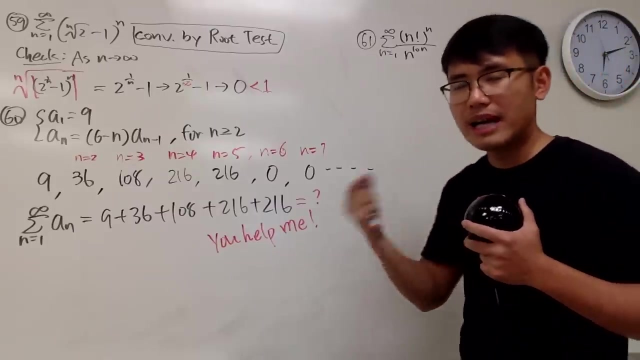 n factorial to the s power, oh my god. n factorial to the nth power over n to the 10 nth power. god, whoa. well, we have the power that has n. so let's do the root test. it's just like that. so here we go, let's go check. 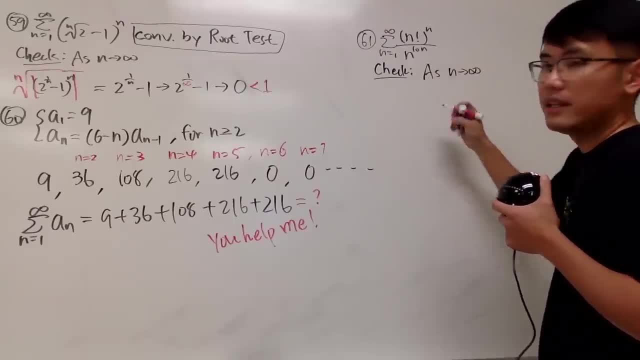 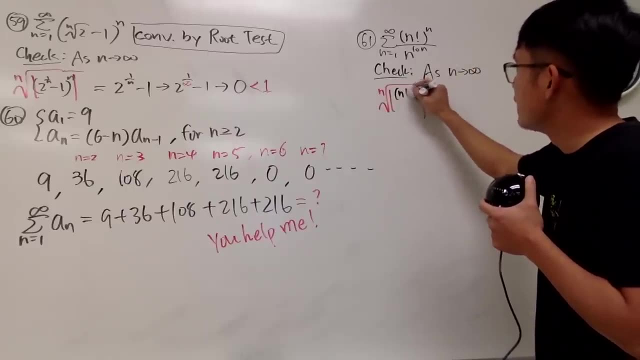 as n goes to infinity. here i'm just going to take the nth root, absolute value, and here we have n factorial, n factorial to the nth power, over n to the 10 nth power. god, and you raise that to the nth power, which is like humongous. 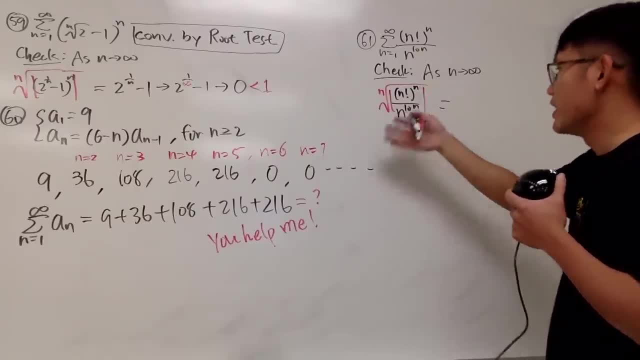 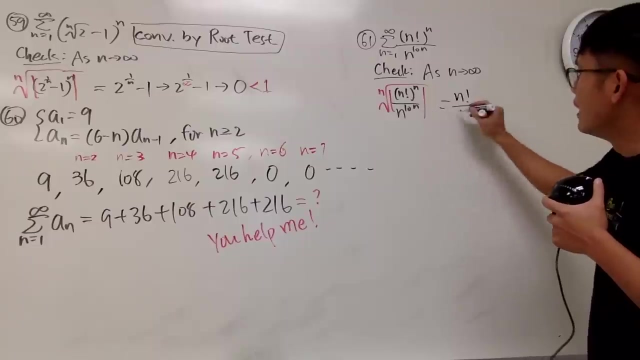 anyway, n and n will be gone, because you are dividing it by because of the root and then the absolute value doesn't make, doesn't, doesn't, doesn't do anything anymore, doesn't matter. anyway. here we have n factorial over n to the 10th power. so what's the conclusion for this guy? 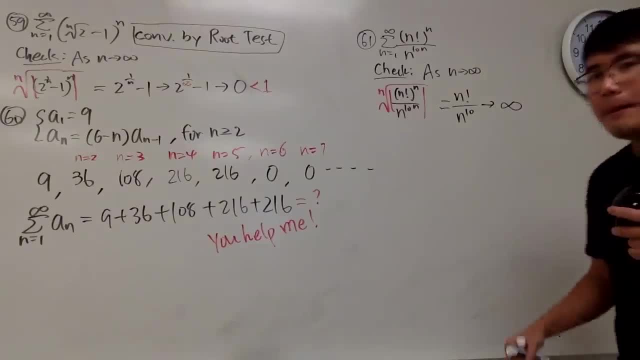 it goes to infinity, because this right here is so much bigger than the nth power one. that means that this right here is even the bottom one. why? how do we know this right here is by the. this right, this right here, prap, you don't want this bigger than 1. 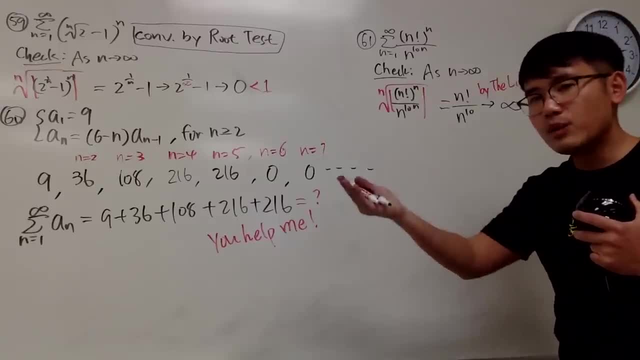 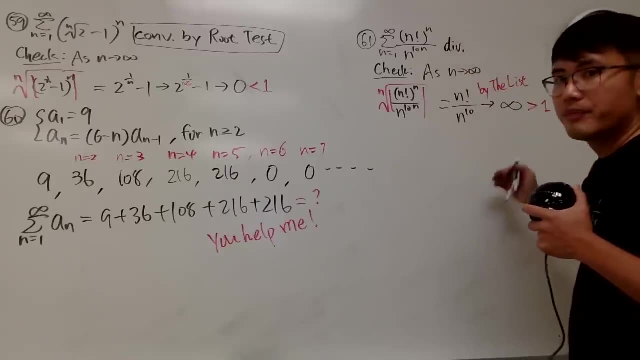 this ⓱ is bigger than 1. we are doing the root test. you have to look at this right here and competitive with one. it's either bigger than 1 or less than what. if it's bigger than one, we can draw conclusion that this right here, actually. diverges your warenasballo to something else. if you want this, than one converges. the last than boiling up is: if Ohio lessons, well, then will здесь alip wieisation. one converges. you have to take into account basically, which is if you only want one but n, or reward nobody, no matter what. 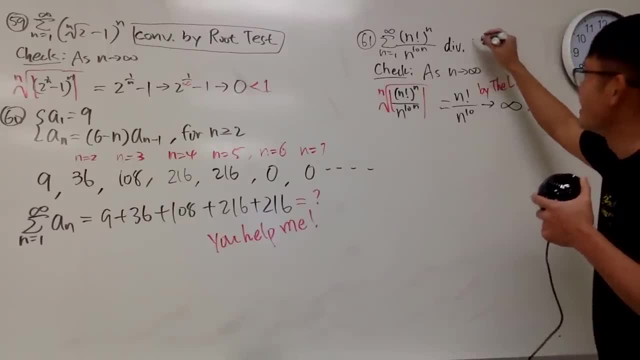 whether you're gonna work or work, at the end of it they will all die, each other two or re- dedans ret utilizar preferred, Unfortunately. try again. right, You have to try again Anyway, by the root test, Like that, Okay. 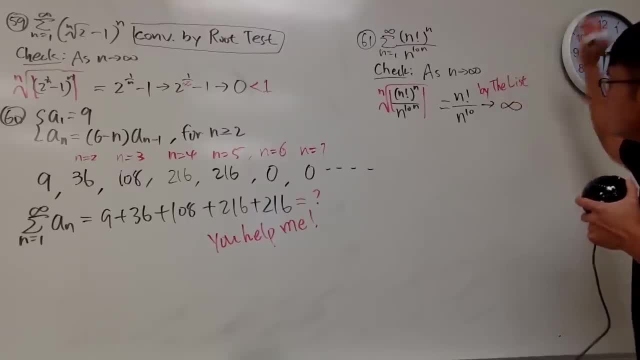 This right here is by the list right. So this right here is, you know, going to infinity. This right here is bigger than 1.. We are doing the root test. You have to look at this right here and compare it with 1.. 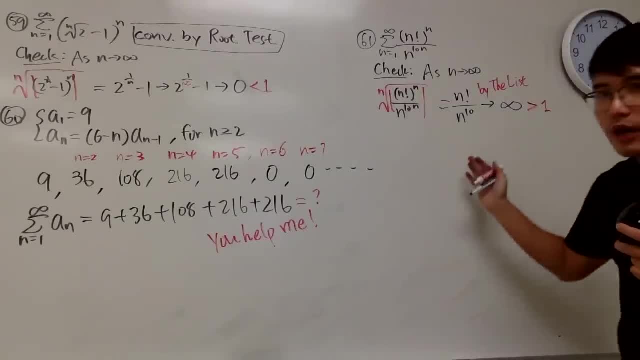 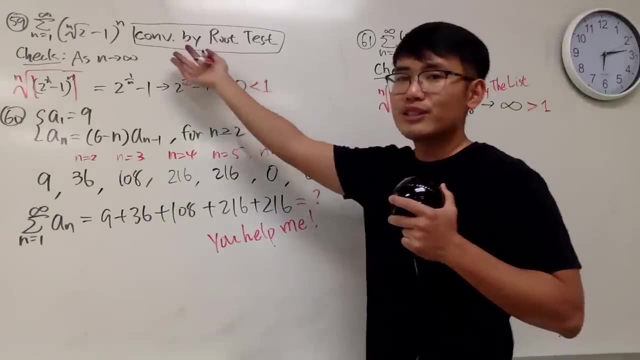 It's either bigger than 1 or less than 1.. If it's bigger than 1, we can draw a conclusion that this right here actually diverges. If it was less than 1, it converges. If it's equal to 1,, unfortunately, we try again, right. 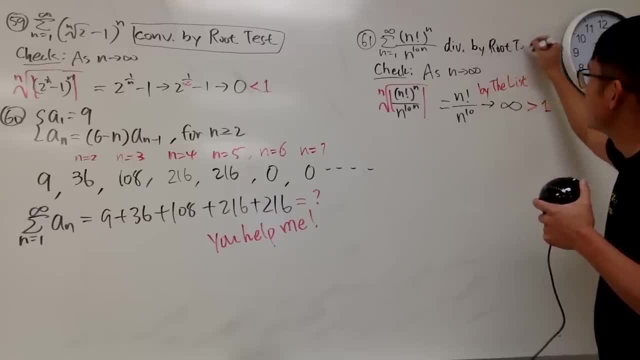 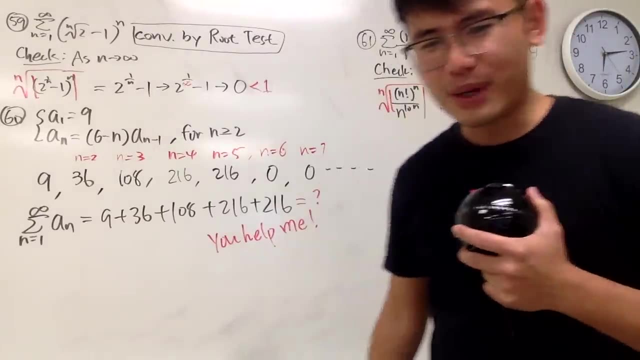 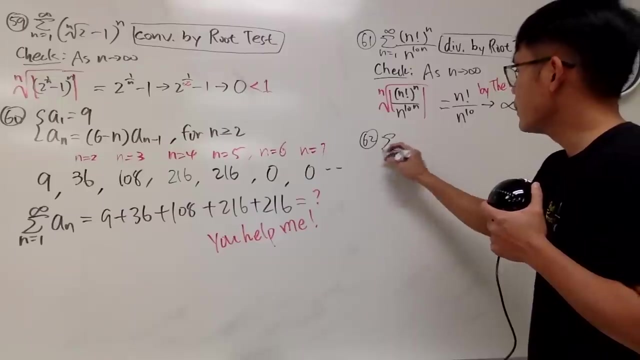 You have to try again, Anyway, by the root test, Like that: Okay, 2n, factorial, 2n, factorial. let's see: Okay, number 62.. Here we go. The sum as n goes from 1 to infinity, parenthesis 2n and then factorial. 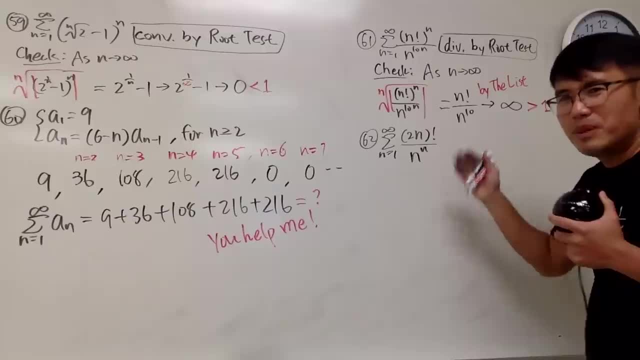 Because you know n to the n is the biggest, but if you have 2n inside here maybe this is some kind of competition. So we'll see. Come on factorial. and then n to the nth, so we'll use the ratio test. 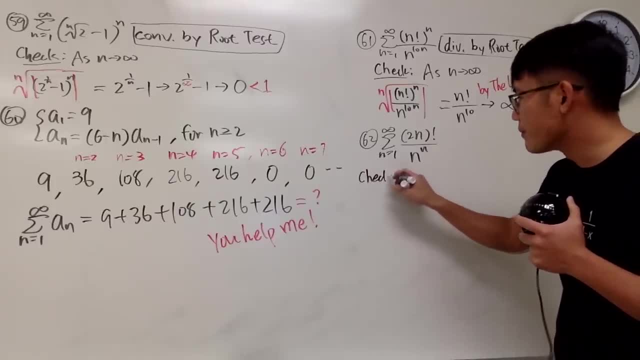 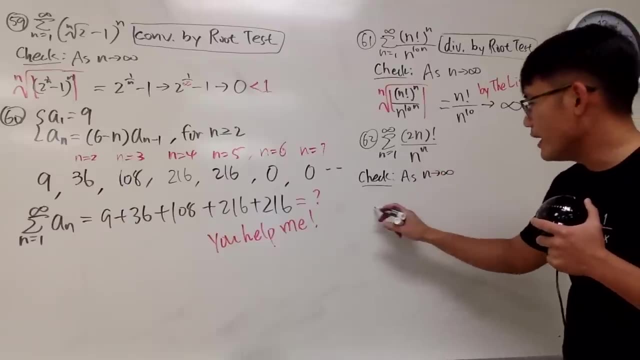 Hmm, So here we go. We're going to do the check again. So check As n goes to infinity, putting n plus 1 into all the n, so we get parenthesis. Oh, I'll take that up for you. And then you have the 2 parenthesis, n plus 1, like this: 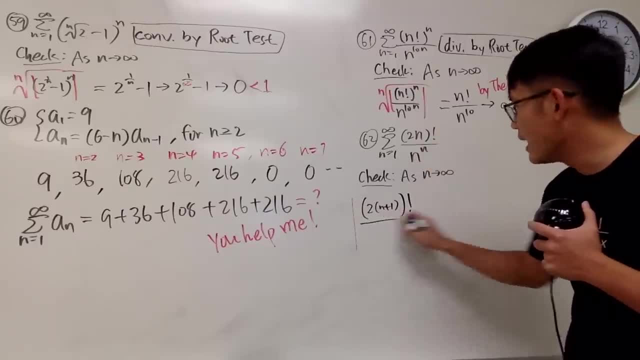 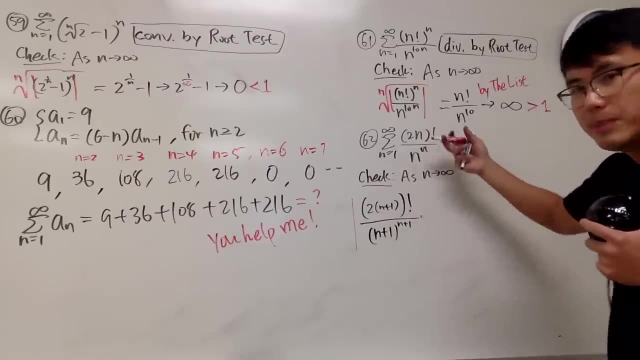 And then the factorial is on the whole side like that, okay, And then divide it by n plus 1, raised to the n plus 1 power, and you multiply it by the reciprocal of the original, so we get n to the n over 2.. 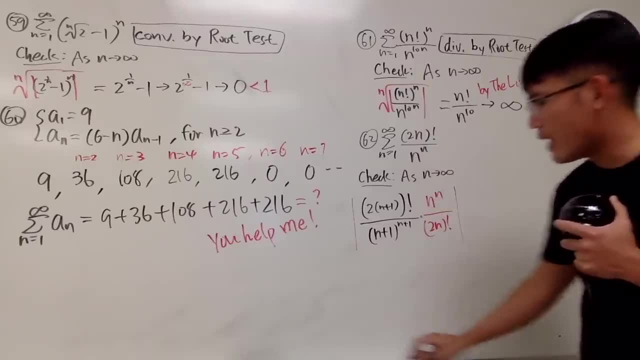 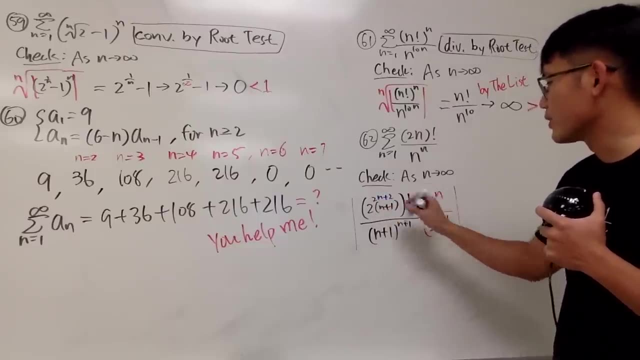 So we have 2n parenthesis and you have the factorial right here. Now here is the DL. Of course, this right here is just 2n plus 2, right, And then you do the factorial. So you get 2n plus 2 times 2n plus 1 times 2n and then you factorial that guy. 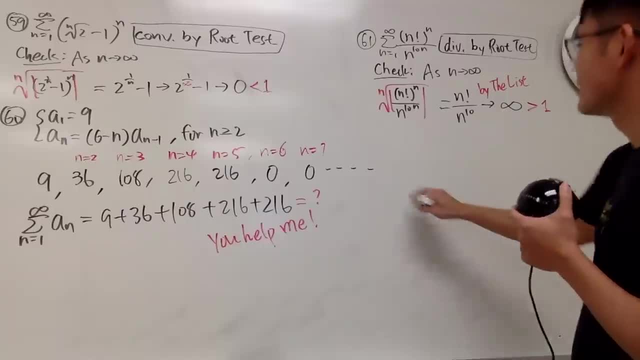 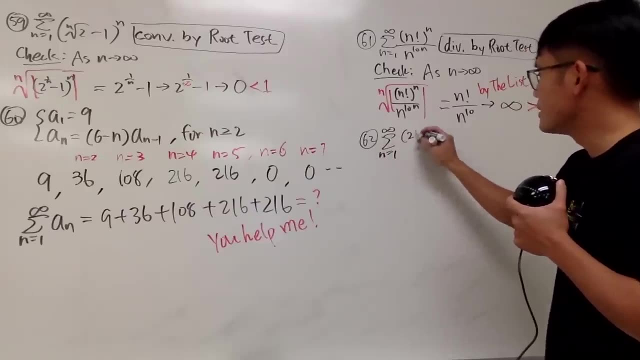 2n, factorial, 2n, factorial. let's see, Okay, number 62.. Here we go. The sum as n goes from 1 to infinity, Parenthesis 2n and then factorial, Because you know, n to the n is the biggest. 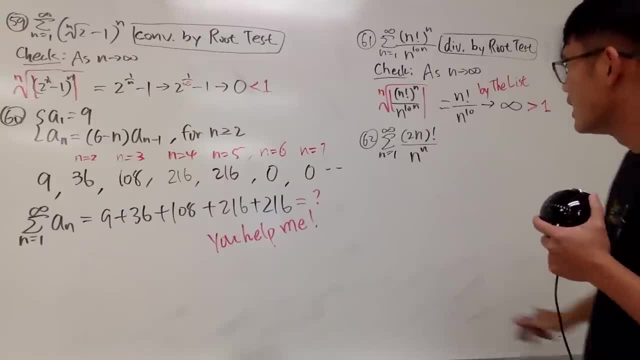 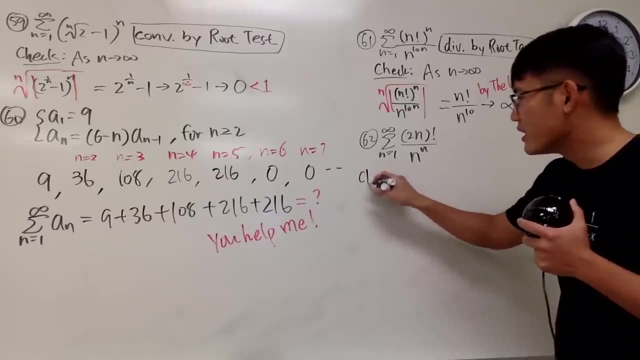 but if you have 2n inside here, maybe this is some kind of competition. so we'll see. Come factorial and then n to the n, so we'll use the ratio test. So here we go. We're going to do the check again. 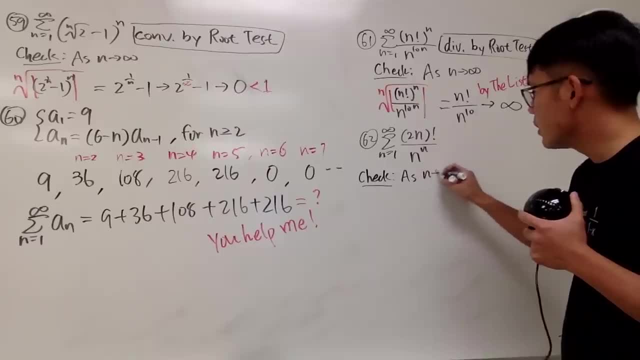 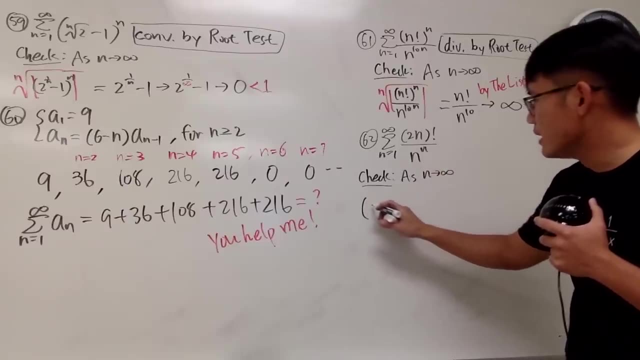 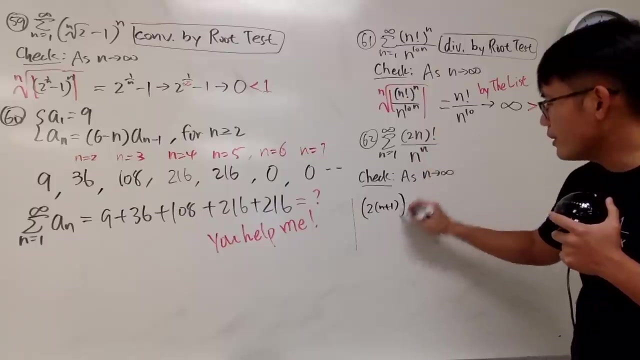 So check s n goes to infinity, Putting n plus 1 into all the n, so we get parentheses- I'll take that for you- And then you have the 2 parentheses, n plus 1, like this, And then the factorial is on the whole side. 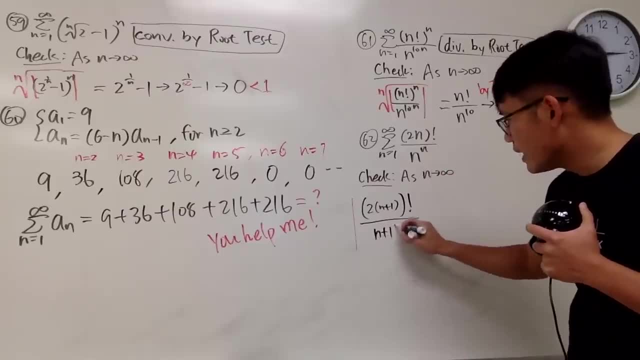 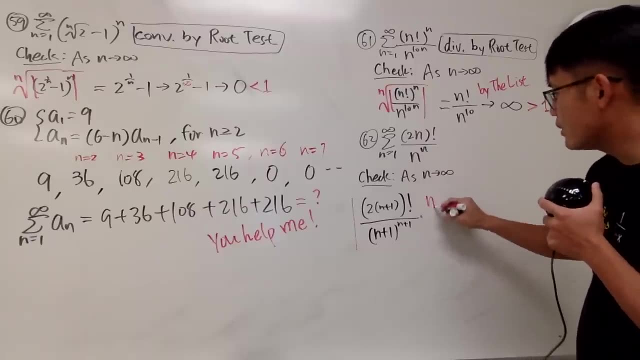 like that. okay, And then divide it by n plus 1, raised to the n plus 1 power, and you multiply it by the reciprocal of the original. So we get n to the n over 2n parentheses and you have the factorial right here. 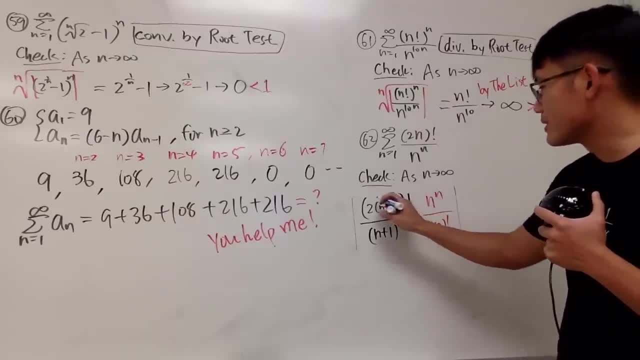 Now here is the deal. Of course, this right here is just 2n plus 2, right, And then you do the factorial, So you get 2n plus 2 times 2n plus 1 times 2n. 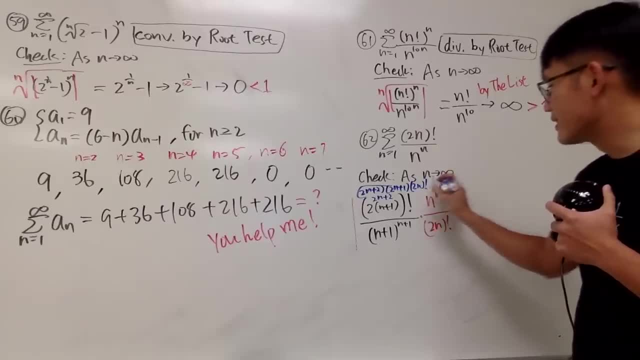 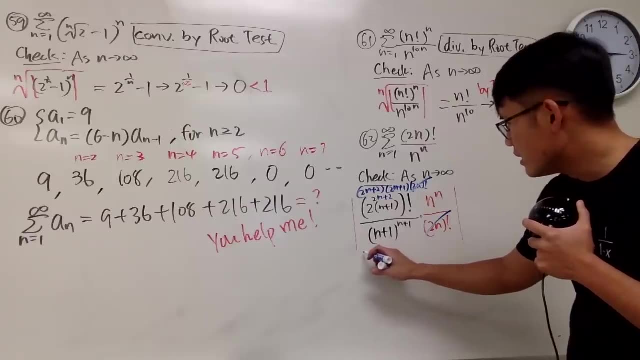 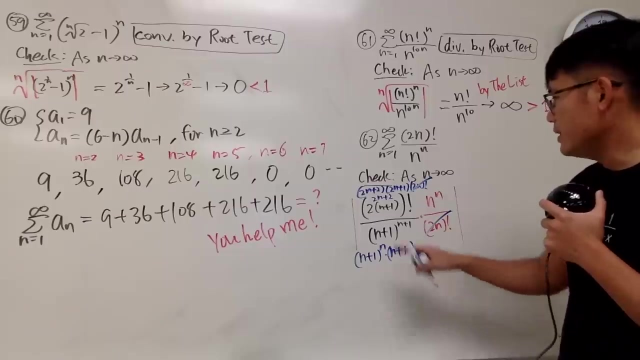 and then you factorial that guy, This guy and that guy cancel out. Now, if you look at this guy, this is the same as saying n plus 1 to the nth power times: n plus 1, like this: And the beauty is that we can factor out a 2.. 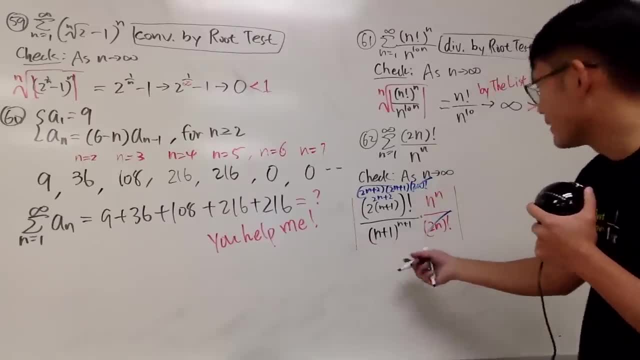 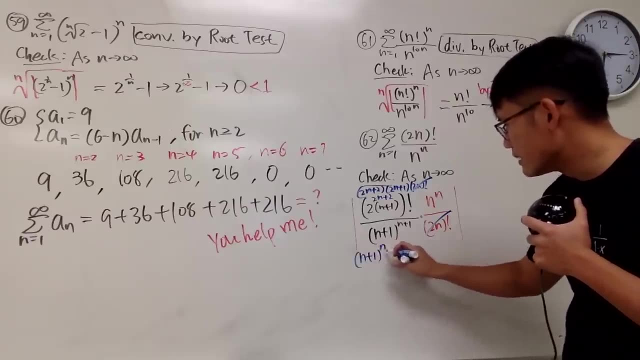 This guy and that guy cancel out. Now, if you look at this guy, this is the same as saying n plus 1.. 2n's power times: n plus 1, like this, And the beauty is that we can factor out a 2.. 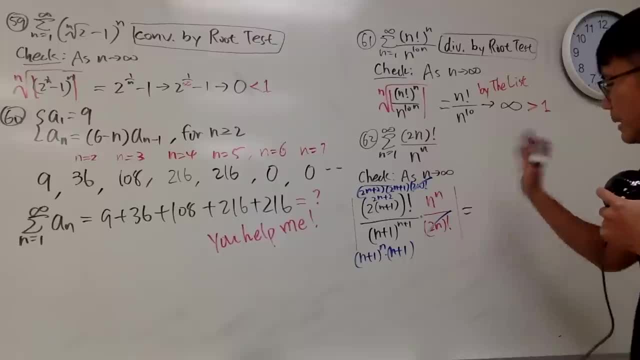 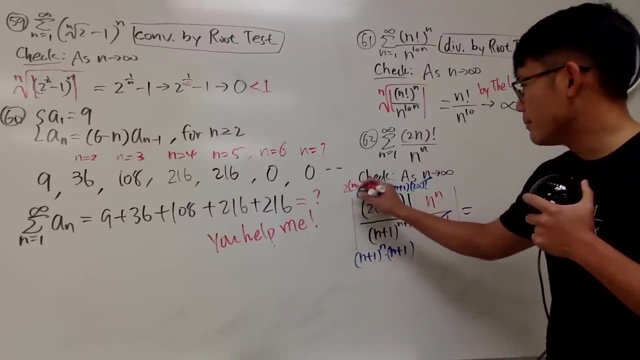 So I'm about to run out of space, so I will probably do that right here. The absolute value doesn't matter, So actually let me just do it over here. This guy is just 2n plus 1, right. So this guy, this is no longer here. 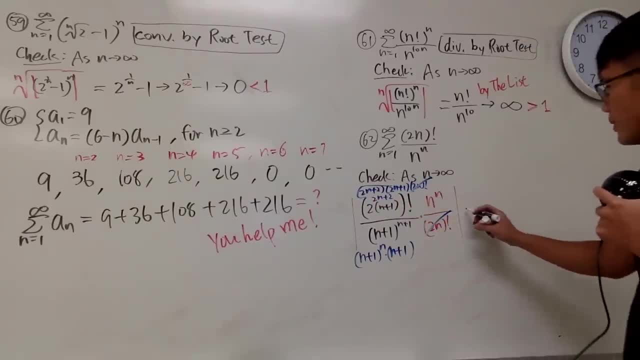 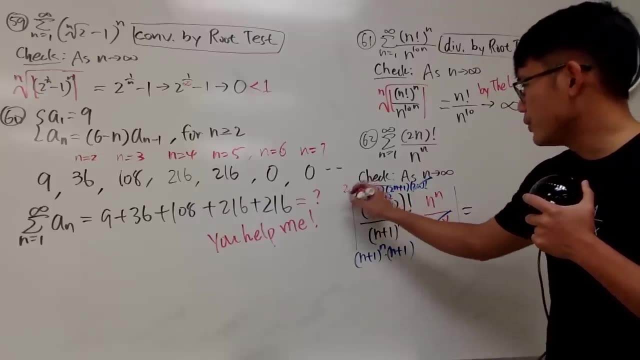 So I'm about to run out of space, so I will probably do that right here. The absolute value doesn't matter, So actually let me just do it over here. This guy is just 2n plus 1, right. 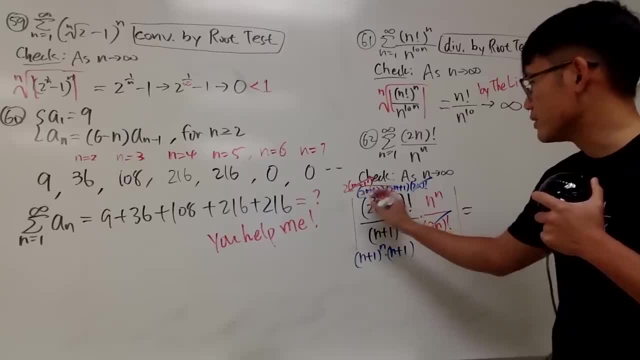 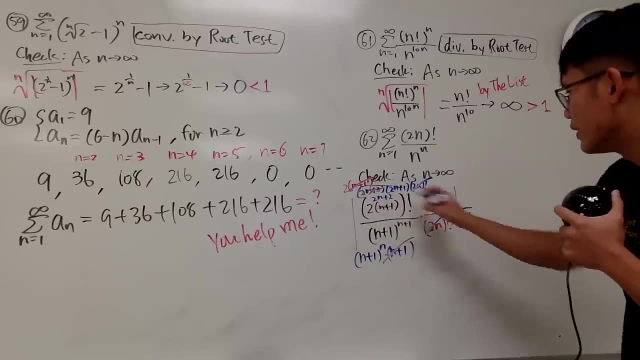 So this guy is just 2n plus 1, right. So this guy is just 2n plus 1, right. So this guy, so this is no longer here. This guy and that guy can be canceled right Now. on the top we have 2 and then 2n plus 1, right. 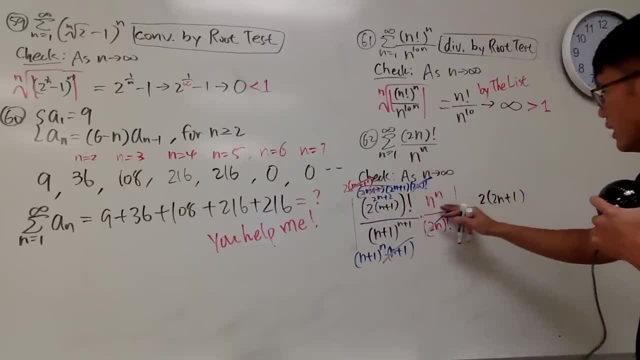 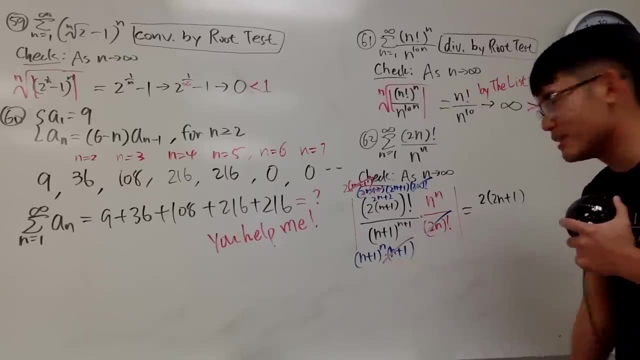 2,, 2n plus 1, and also n to the nth power. okay, Okay, But I feel like I have to do something with this again. by the limit, We did the equation earlier, So I will just write it down nicely like this: 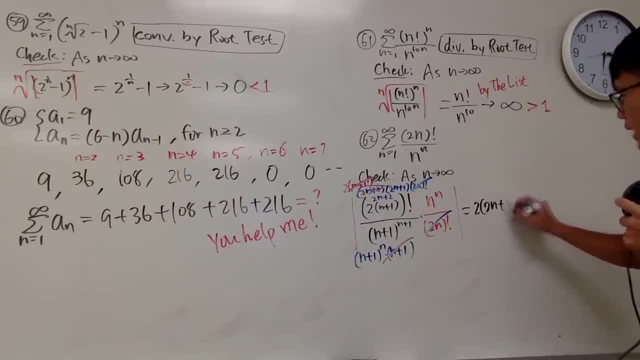 2, 2n plus 1.. 2, 2n plus 1, like that. So put that down first and this over that. So I just multiply by n to the n over n plus 1 to the nth power. 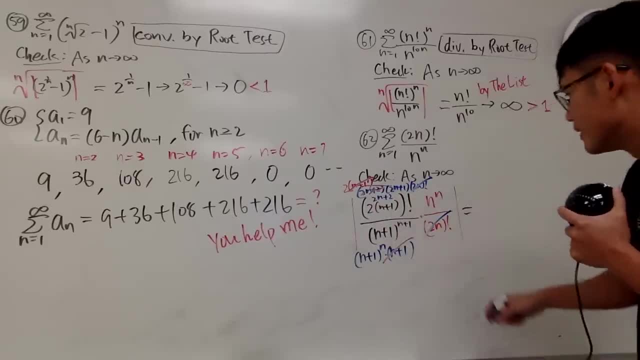 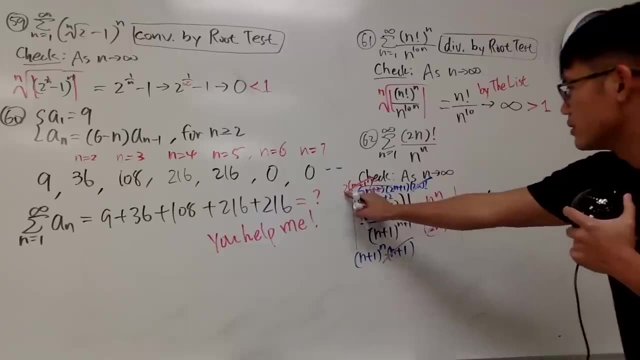 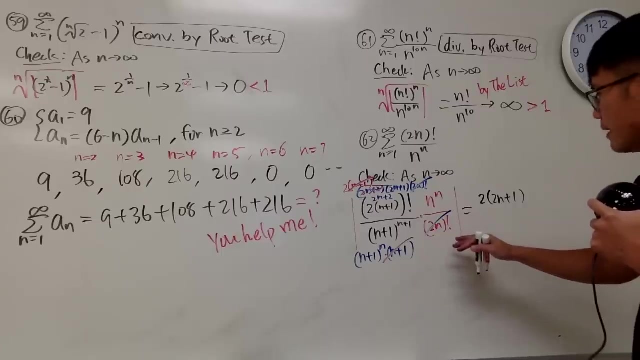 This guy and that guy can be canceled right Now. on the top we have 2, and then 2n plus 1.. 2n plus 1 and also n to the nth power. okay, But I feel like I have to do something with this again by the limit. 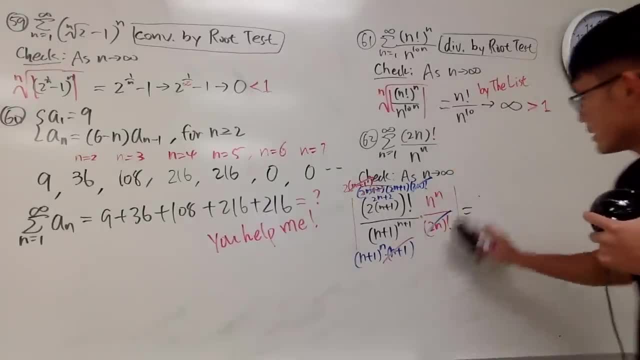 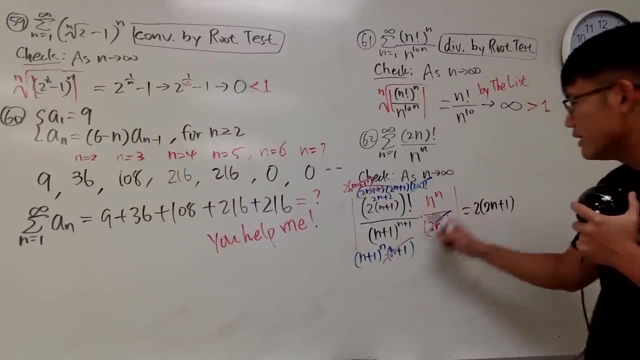 We did the equation earlier, So I will just write it down nicely like this: 2, 2n plus 1, like that. So put that down first and this over that. So I just multiply by n to the n over n, plus 1 to the nth power. 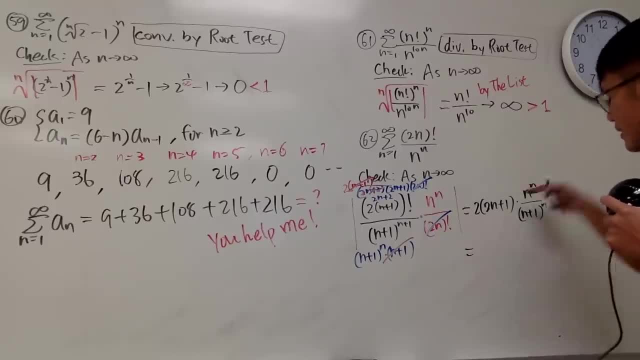 So how did we do this earlier? Well, we factor out the n to the power, right? Just bring that out. So if you want, you can just distribute this to be Q a little bit. This is 4n plus 2 times this. right here is just n over n plus 1 raised to the nth power. 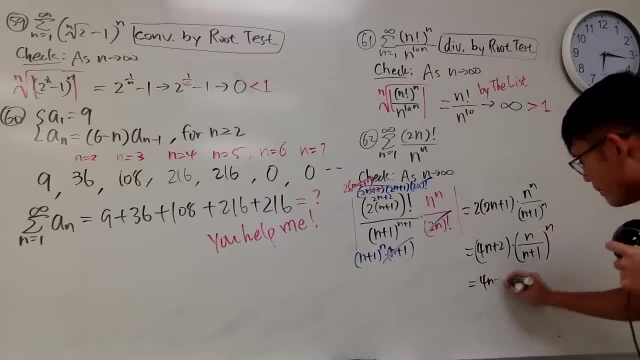 Flip this, make that into negative. So this is 4n plus 2 times this right here inside is n plus 1 over n And you make this into negative exponent Right. And now you see this right here is equal to 4n plus 2 times this guy is 1 plus 1 over n, raised to the negative nth power. 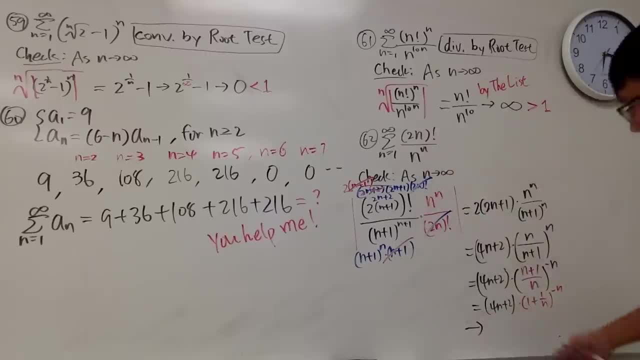 Now take the limit, as n goes to infinity. The first guy actually goes to infinity Times, even though the second guy is nicely behaved. you use the fact you get 1 over e, But infinity is so much bigger compared to e. 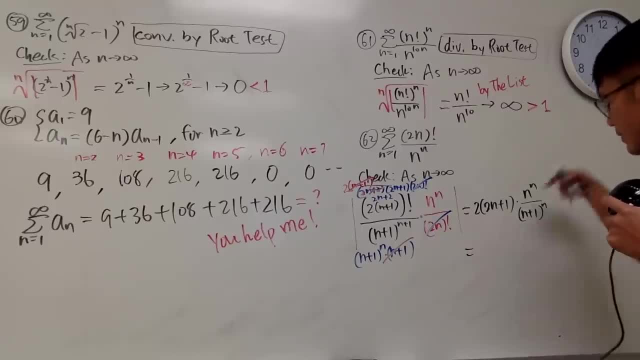 So how did we do this earlier? Well, we factor out the n to the power, right? Just bring that out. So if you want, you can just distribute this to be cute a little bit. This is 4n plus 2 times this. right here is just n over n plus 1 raised to the nth power. 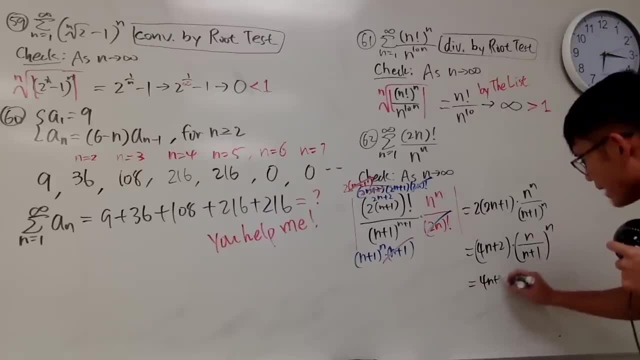 Flip this. This is n to the negative. so this is 4n plus 2 times this right here inside is n plus 1 over n and you make this into negative exponent right. And now you see this right here is equal to 4n plus 2 times this guy is 1 plus 1 over n raised to the negative nth power. 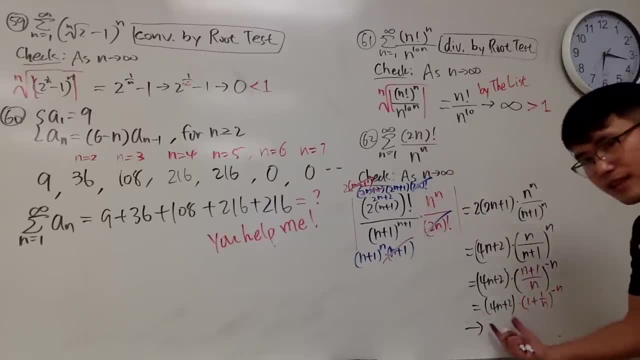 Now take the limit, as n goes to infinity. The first guy actually goes to infinity Times, even though the second guy is nicely behaved. you use the fact you get 1 over e, But infinity is so much bigger compared to e. 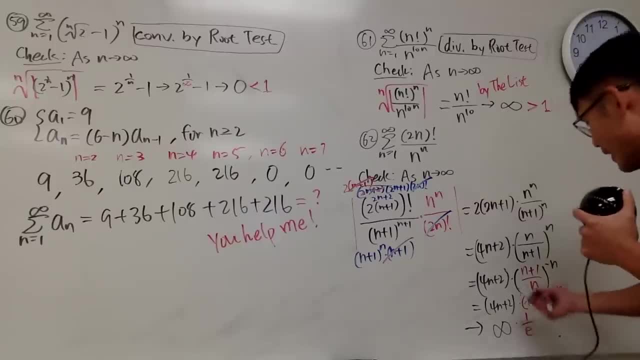 This is like Thanos and this is like Iron Man, right? So you actually still end up with just infinity. If you are doing the ratio test and if you end up with a limit, if this limit is bigger than 1, what can we say? 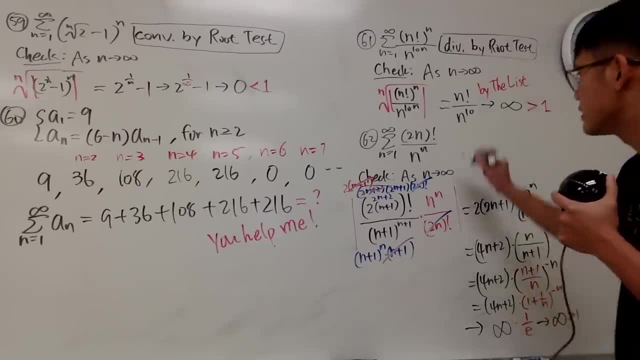 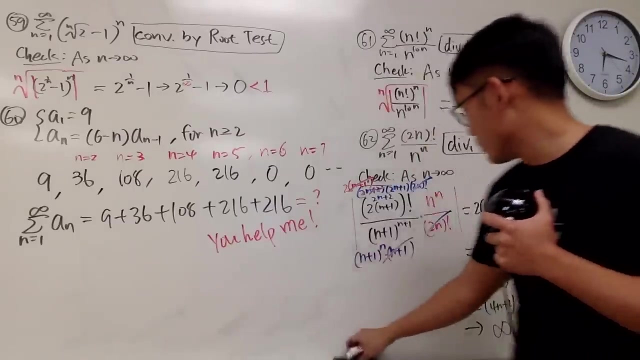 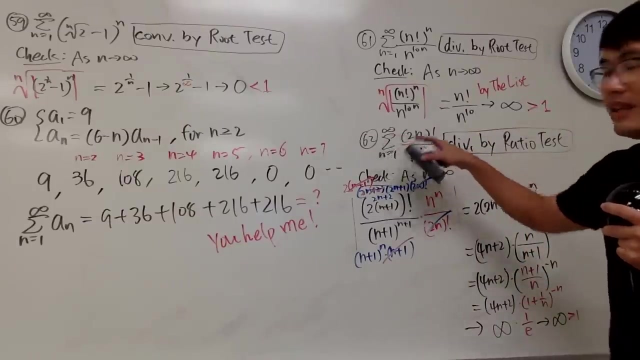 This guy right here- Time purchase By the ratio test. okay, So in fact, the top is actually so much, much more powerful than the bottom. Okay, so that's it. In fact, if you can do the test of divergence, you can also try that. but I will leave that to you guys. 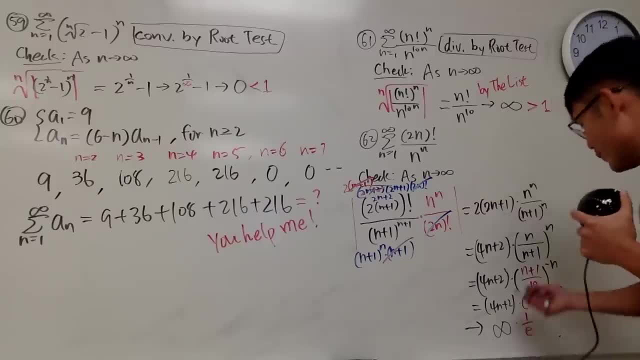 This is like- And this is the element right- So you actually still end up with just infinity. If you're doing the ratio test and if you end up with a limit- if this limit is bigger than 1, what can we say? 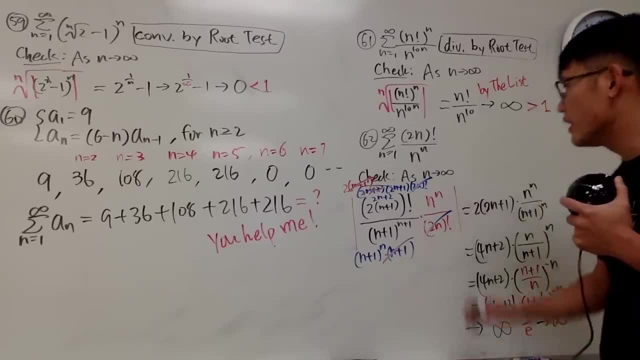 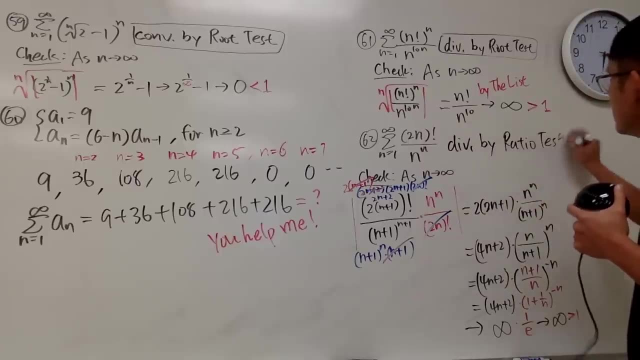 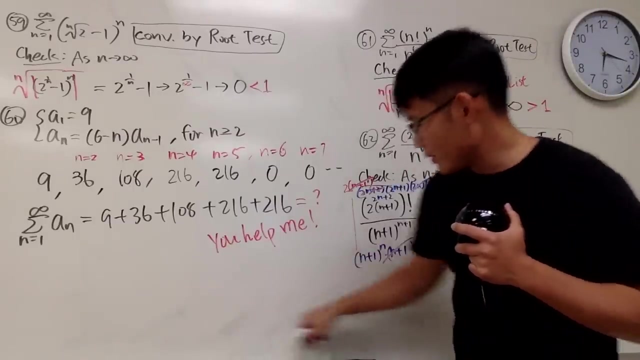 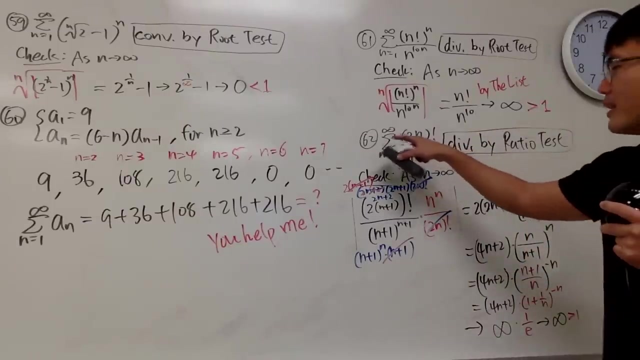 This guy right here- Type purchase by the ratio test. Okay, So in fact, the top is actually So much, much more powerful than the than the bottom. Okay, so that's it. In fact, if you can do the test of divergence, you can also try that too. but I will leave that to you guys. 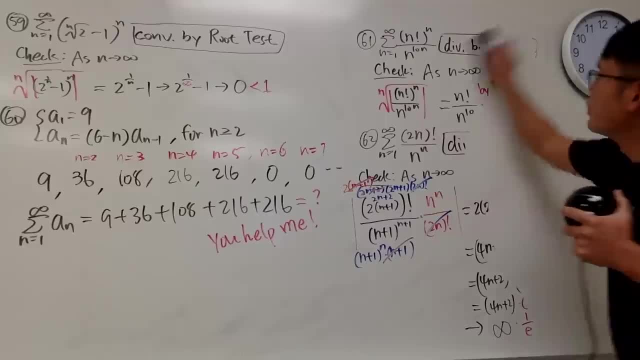 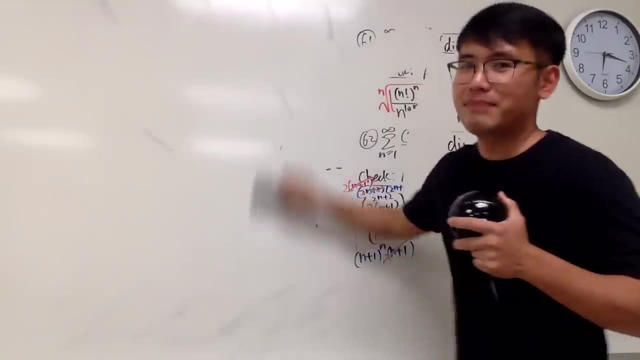 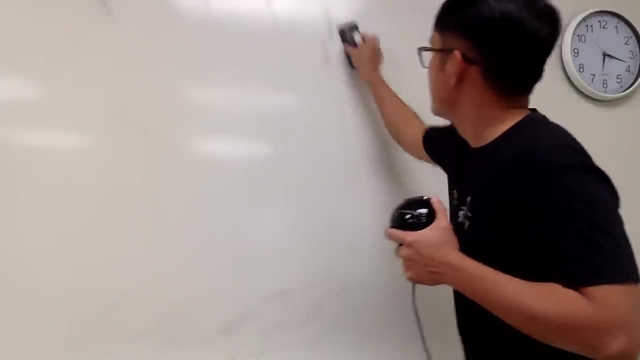 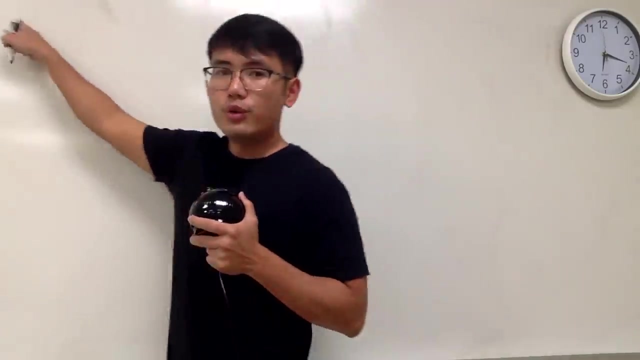 Okay, so that's it for that. Okay, We have a couple more to go, So 62.. This is taking much longer than I was expecting, seriously, But okay, We'll see. Okay. 63, right here. 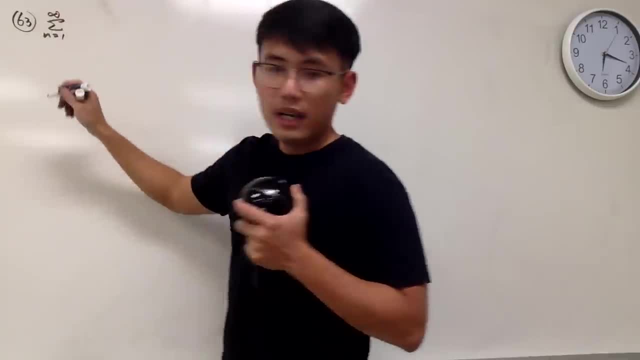 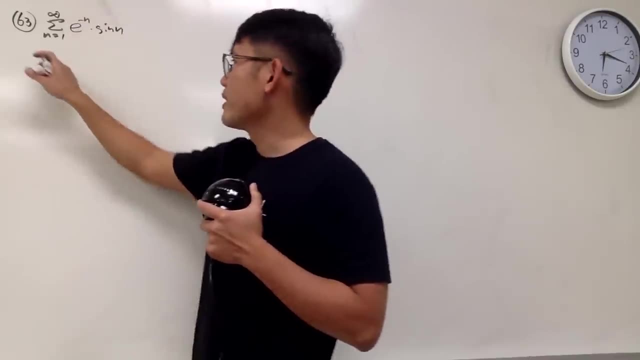 The sum as n goes from 1 to infinity. And here we have e to the negative n. times sine n. Yes, e to the negative n. Bring that down to a denominator. so, if you like, This is the sum as n goes from 1 to the infinity. 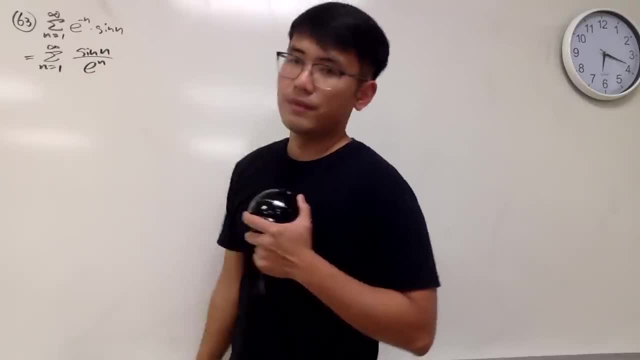 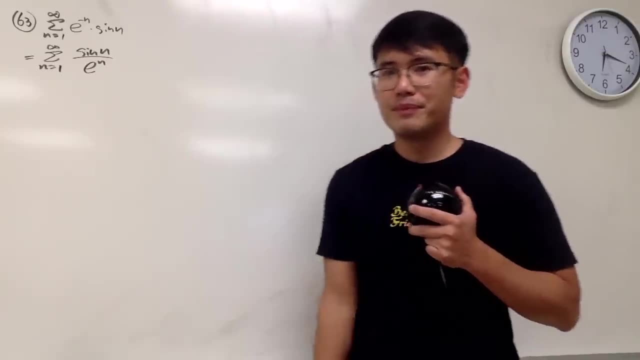 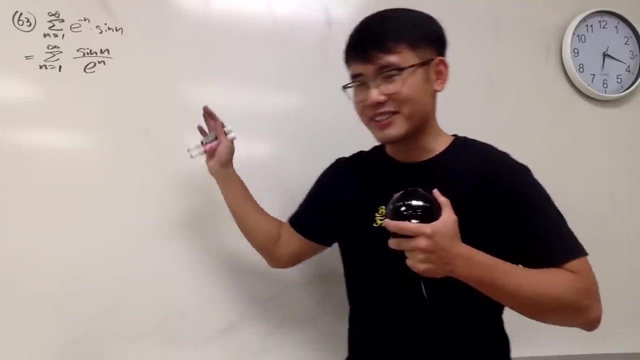 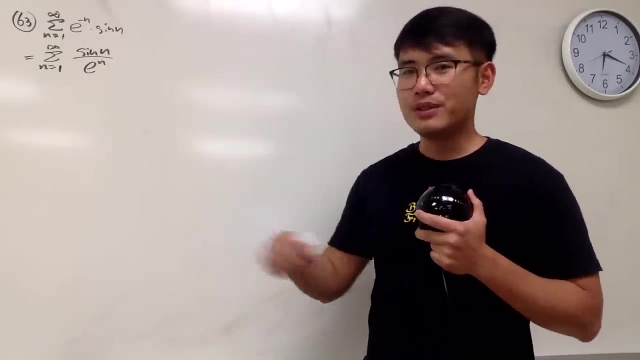 On the top we have sine n over e to the n, Good. Good. Now here is the DEO. Can we use the integral test? No integral test, Anyway, because I'll say that in Chinese, because this right here, um, it's not always positive. so integral test doesn't work and it does not decrease all the time, right? 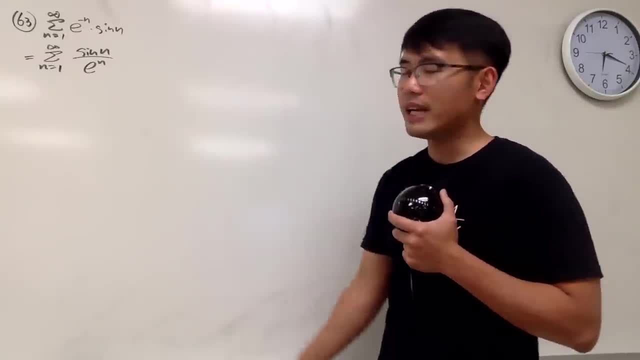 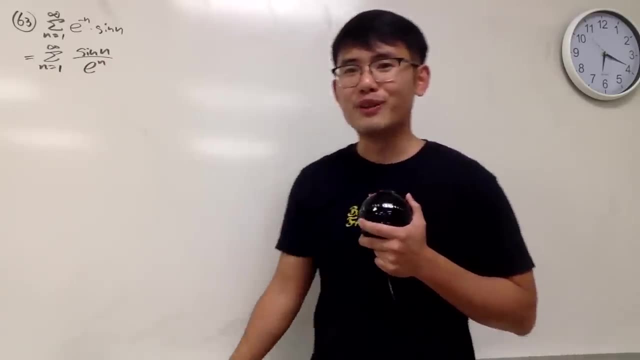 So no, no integral test, even if we can get that. but no, Well, the way to do it is we can just again, we have the sine. So let's check for n, For absolute convergence. So notice the following: 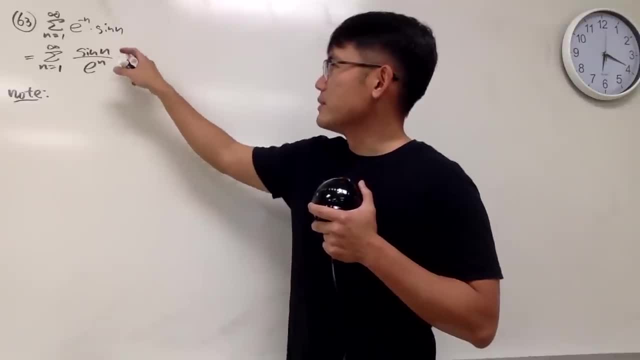 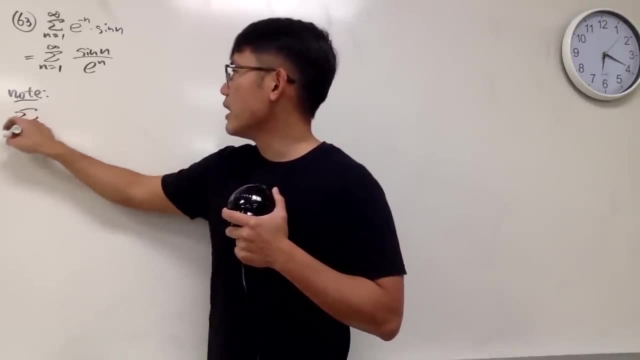 And the truth is I'm not going to just like put on the um inequalities, because this is not always positive, so I really have to take the absolute value and then just talk about how it is in the absolute sense, right here, right? 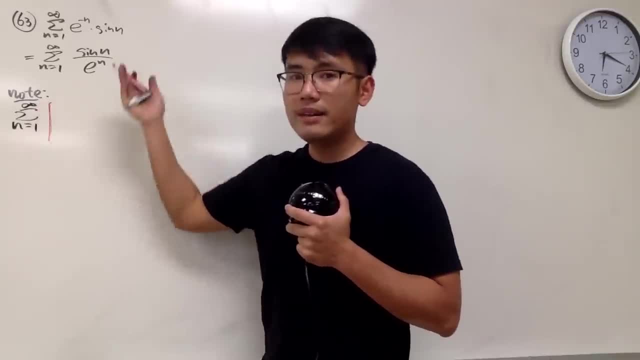 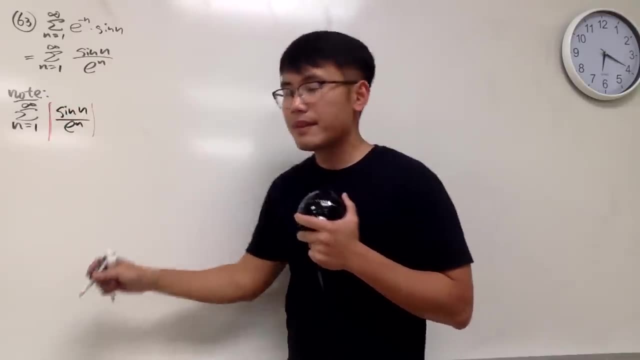 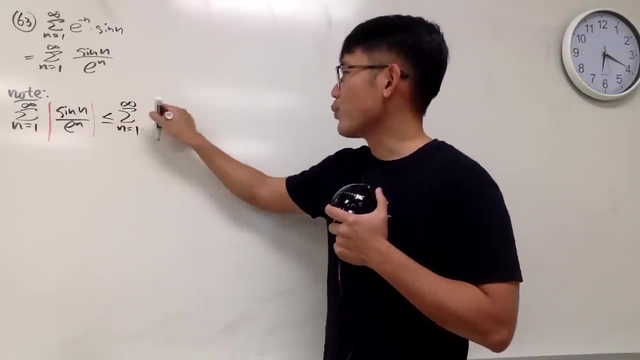 So take the absolute value and on the top we have sine of n over e to the n, like this: Now, thanks to the inequality that we have done so many times so far, we can know that this is one to infinity. on the top, it's just one right. 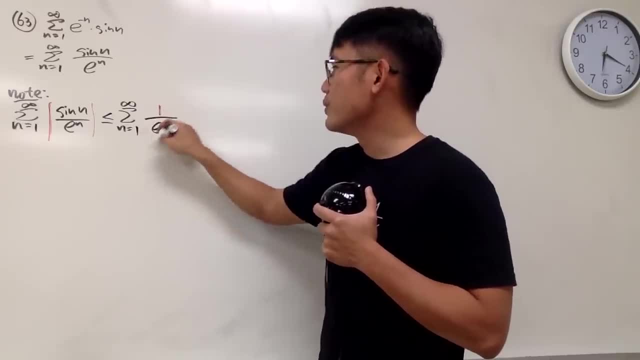 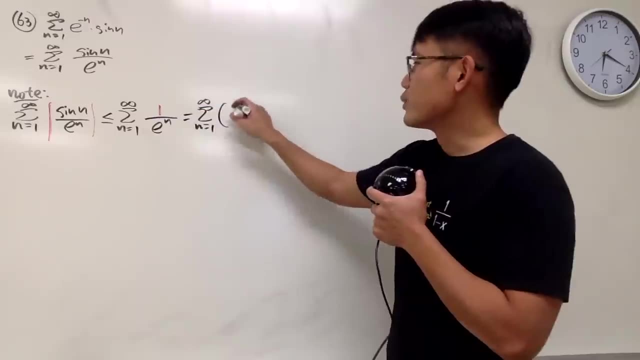 Sine n is always less than or equal to one over e to the n, And this, right here we can rewrite it, Of course. this is the sum, as n goes from one to infinity. This is one over e to the nth power. 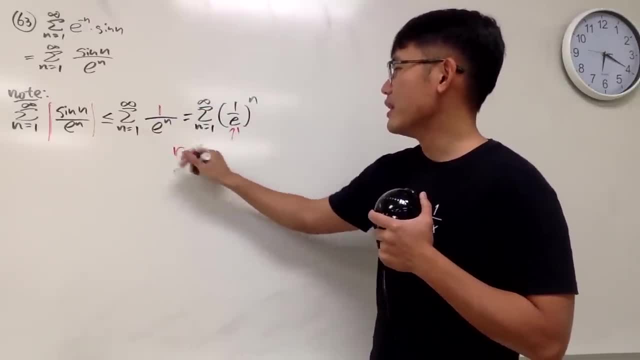 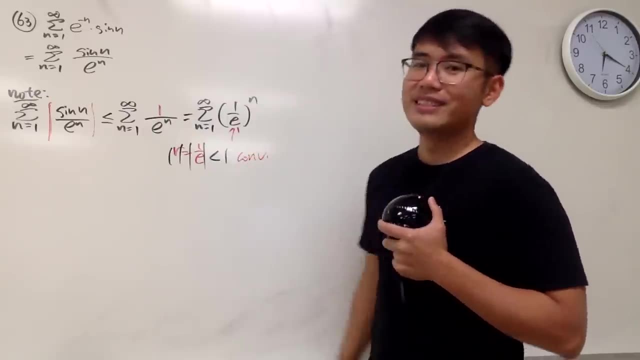 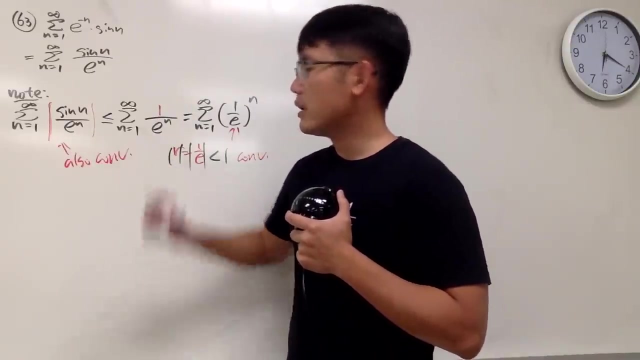 What's this? Yes, r is equal to one over e. Take absolute value. absolute value, This right here is less than one, which is, uh, convergent geometric series, right? So that means this right here also converges. 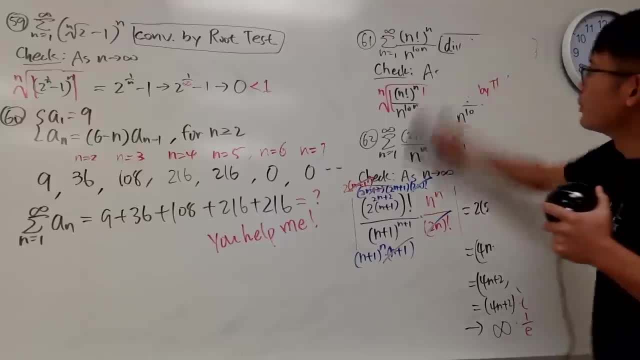 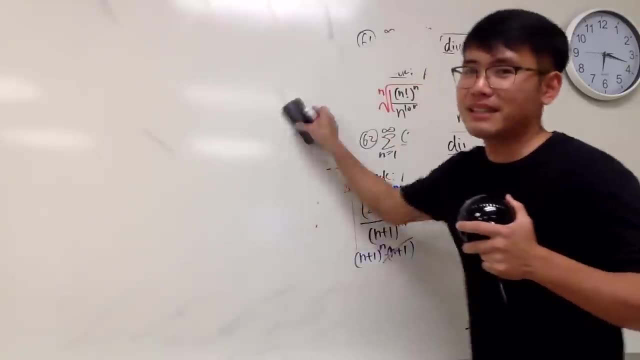 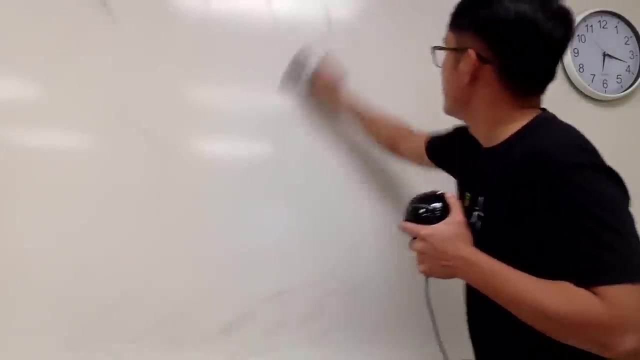 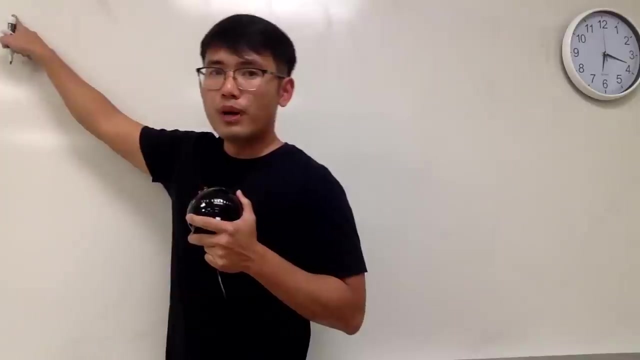 Okay, so that's it for that. Okay, we have a couple more to go, so 62.. This is taking much longer than I was expecting, seriously, But okay, we'll see. Okay, 63 right here. The sum as n goes from 1 to infinity. 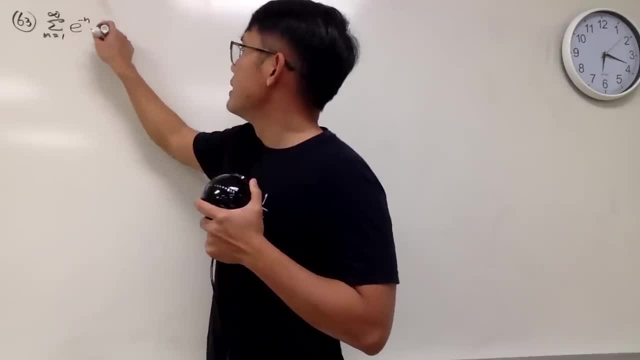 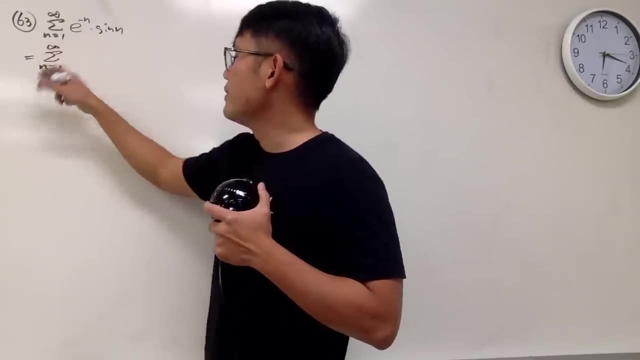 And here we have e to the negative n. times sine n. Yes, e to the negative n. bring that down to a denominator. so, if you like, this is the sum as n goes from 1 to the infinity. On the top we have sine n over e to the n. 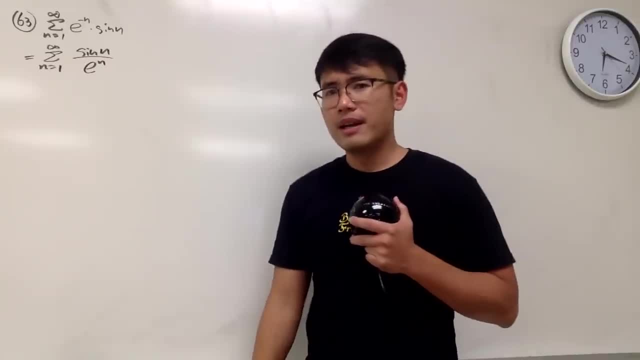 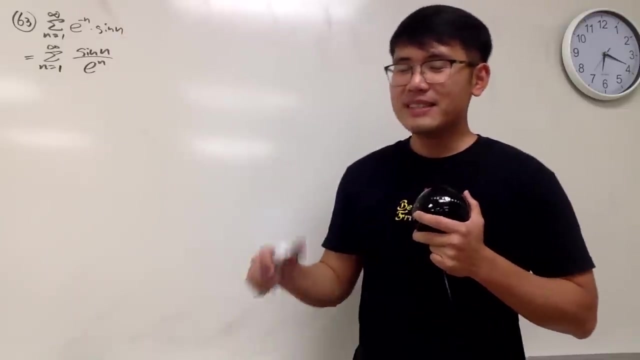 Good, Now here is the DEO. Can we use the integral test? No integral test, Anyway, because I'll say that in Chinese, because this right here, it's not always positive. so integral test doesn't work And it does not decrease all the time, right. 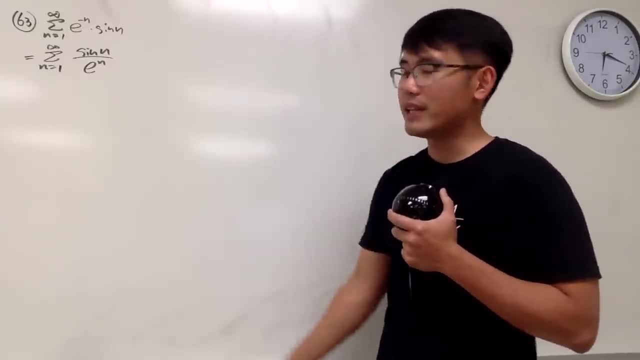 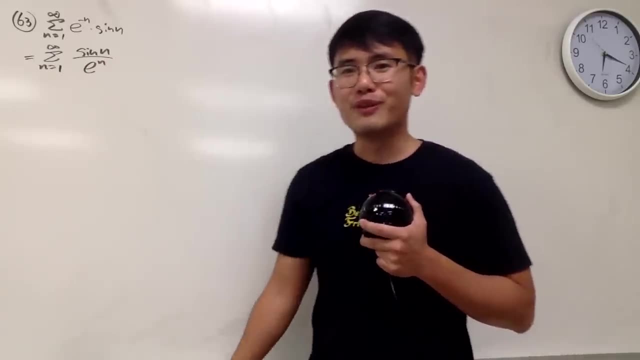 So no integral test, even if you can grade that. but no, Well, the way to do it is we can just again, we have the sine. so let's check for absolute convergence. So notice the following: 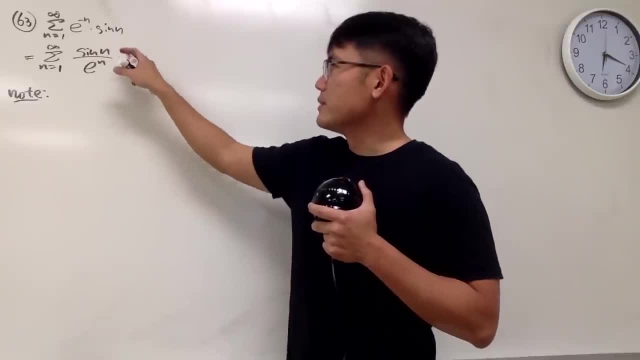 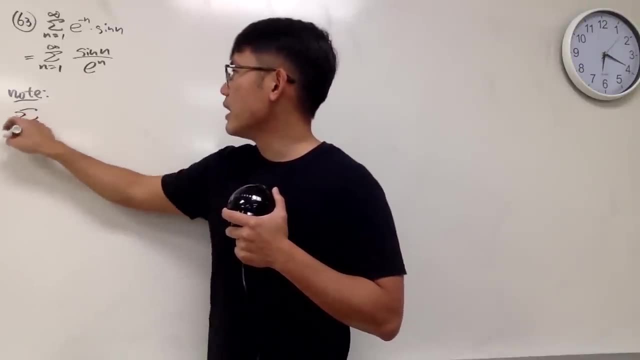 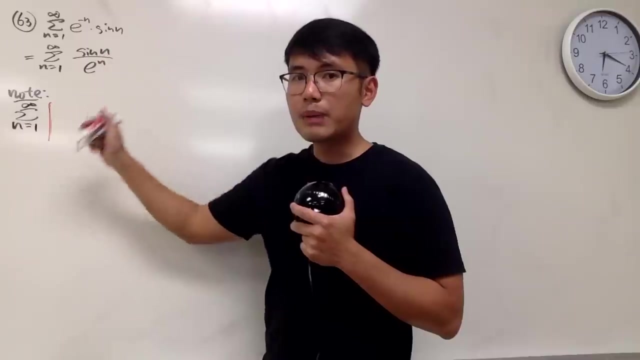 And the truth is I'm not going to just put down the inequalities, because this is not always positive, so I really have to take the absolute value and then just talk about how it is in the absolute. Okay, So let's take the absolute value and on the top we have sine of n over e to the n, like this: 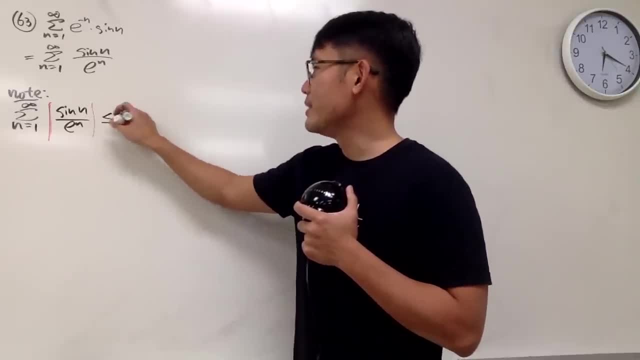 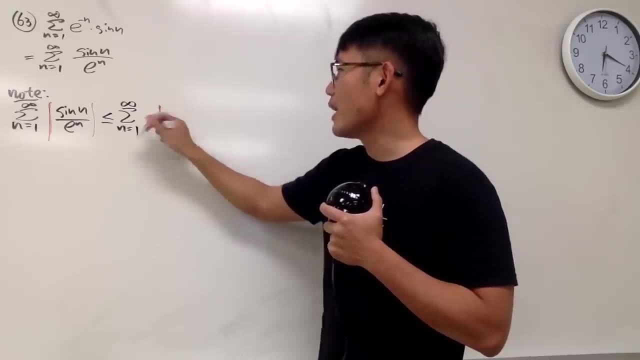 Now, thanks to the inequality that we have done so many times so far, we can know that this is 1 to infinity. On the top it's just 1, right Sine n is always less than or equal to 1. over e to the n. 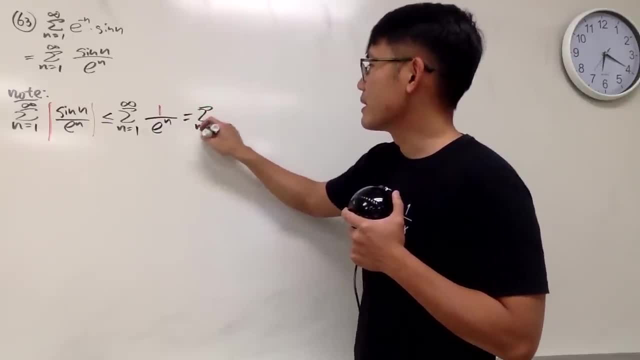 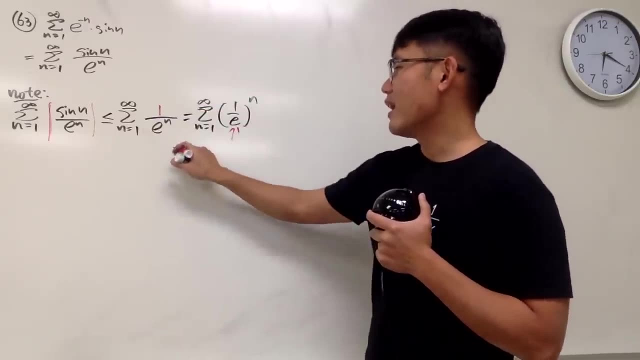 And this right here, we can rewrite it, Of course. this is the sum, as n goes from 1 to infinity. This is 1 over e to the nth power. What's this? Yes, r is equal to 1 over e. 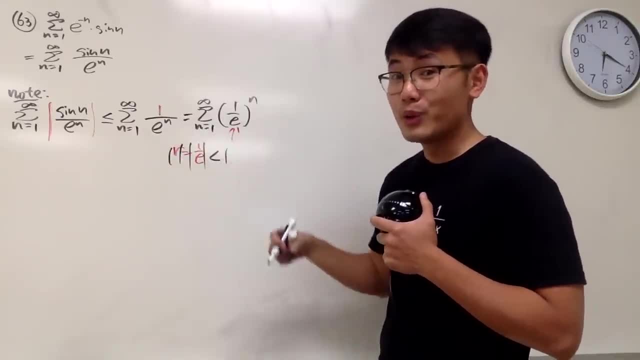 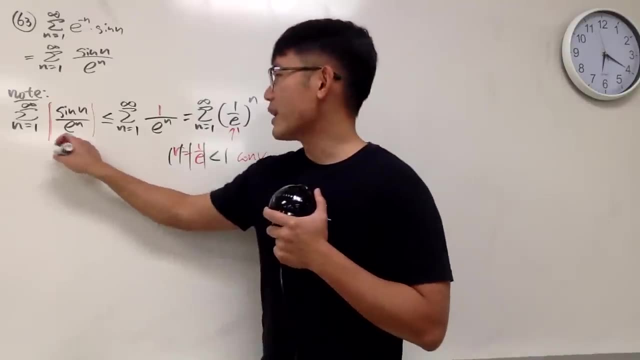 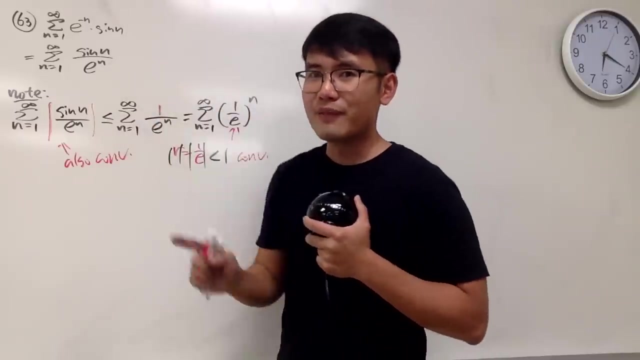 Take absolute value. absolute value, This right here is less than 1, which is convergent geometric series right. So that means this right here also converges. In another word, in fact, this right here converges absolutely, and I will actually come back here and tell you guys, of course, if it converges absolutely. 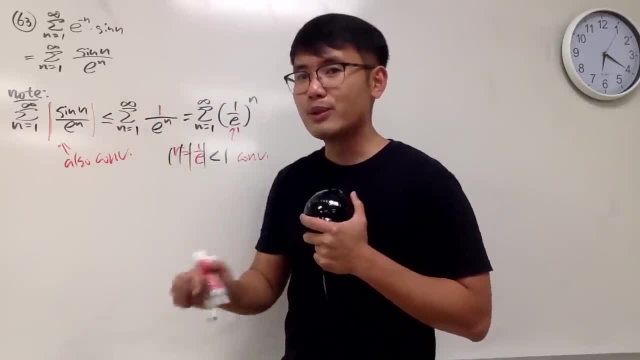 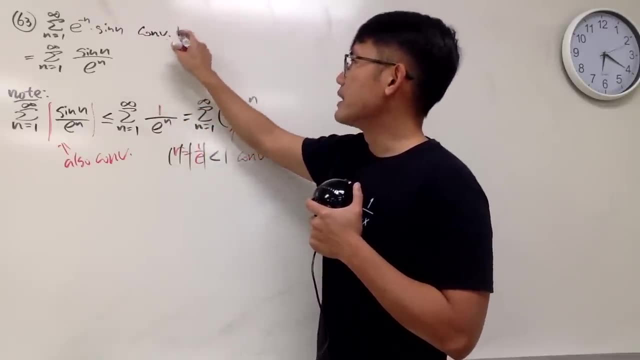 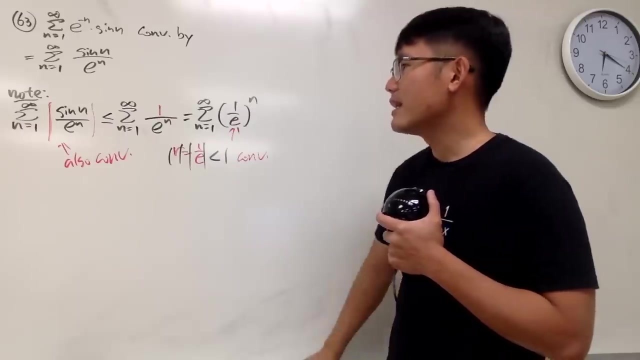 In another word: in fact, this right here converges absolutely, and I will actually come back here and tell you guys, of course, if it converges absolutely, it converges as well, and it's actually by comparison test. I will actually say, hmm, ah, yeah, this is kind of tricky. 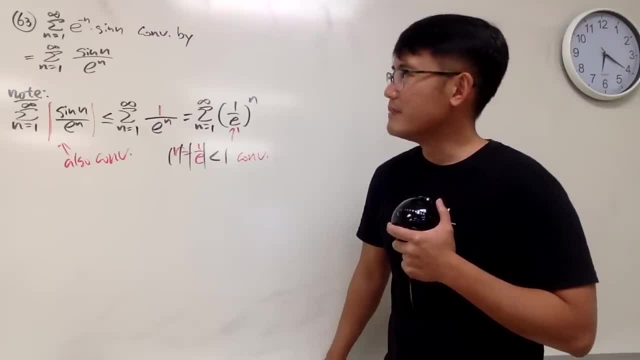 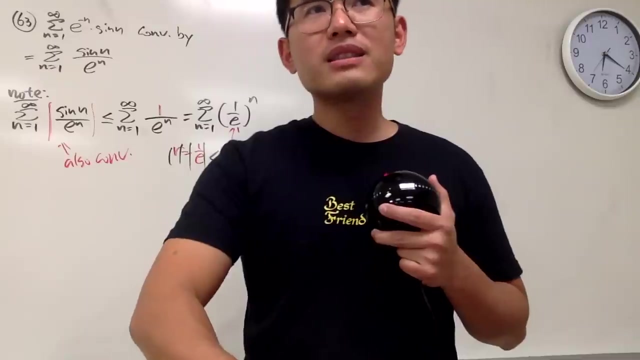 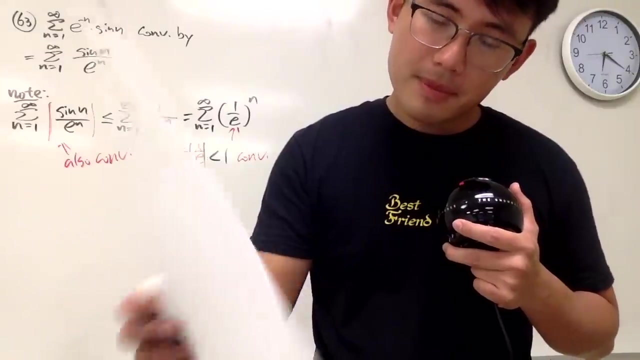 because for comparison test I should have said: oh yeah, that's tricky. Oh man, when I take the absolute value for the cosine 1.. Oh no, that was the alternating, so I was good. Okay, didn't make that mistake earlier. 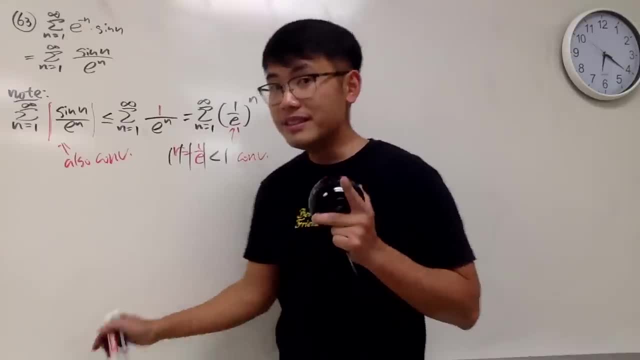 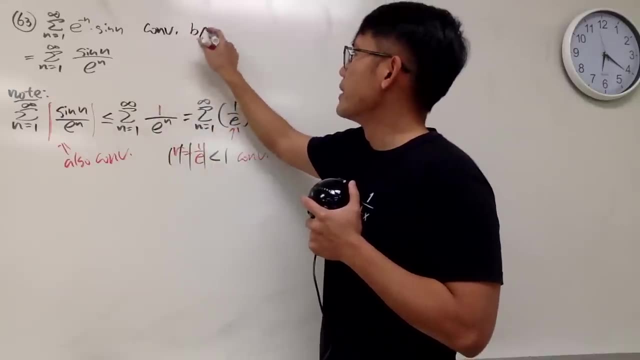 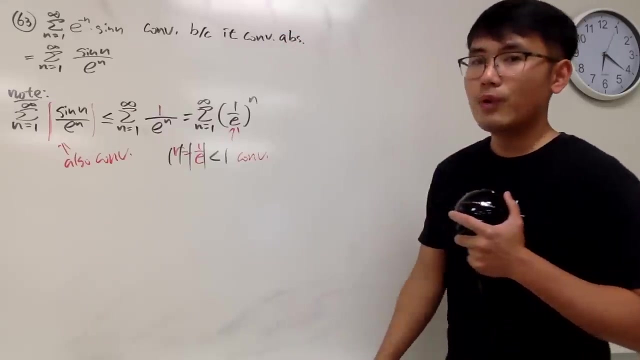 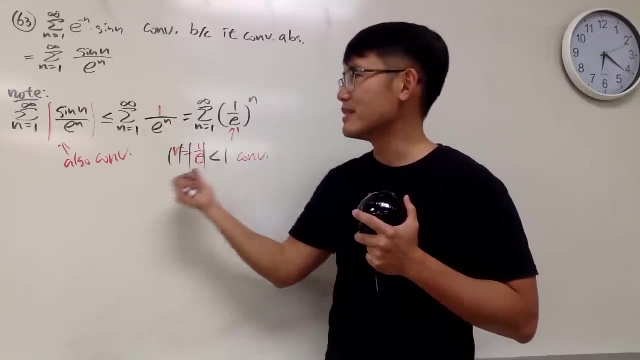 Okay, so here is the DO. This is why that this actually converges. okay, This right here converges. because it converges absolutely. Why? Because the absolute version right here, based on the comparison test, it works. Based on the comparison test, it works. 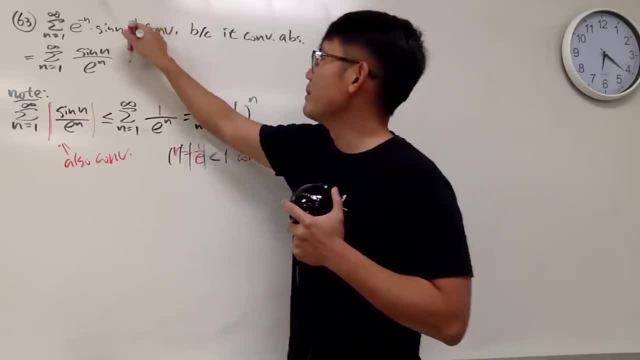 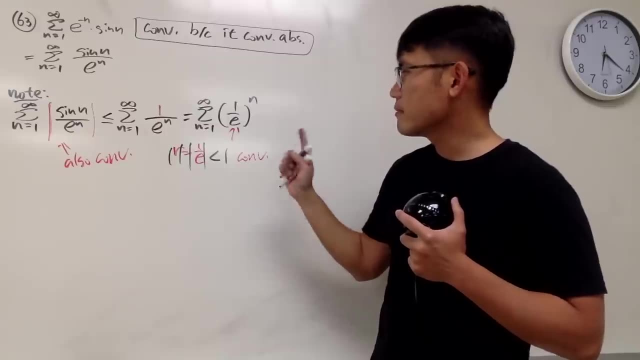 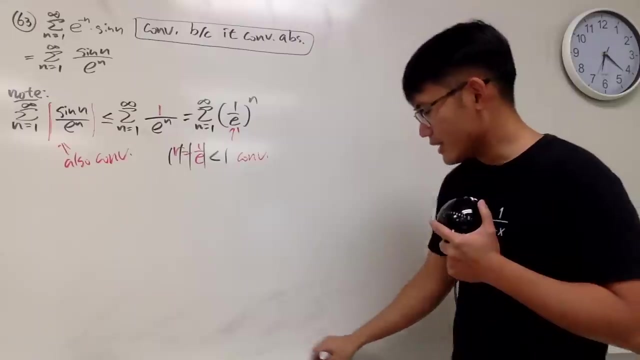 And yeah, Yeah, It converges absolutely. because it converges absolutely and the absolute value version, this right here is the when, this, when everything is positive, you can do the comparison test. So that kind of reminds me of the question that we did like earlier. 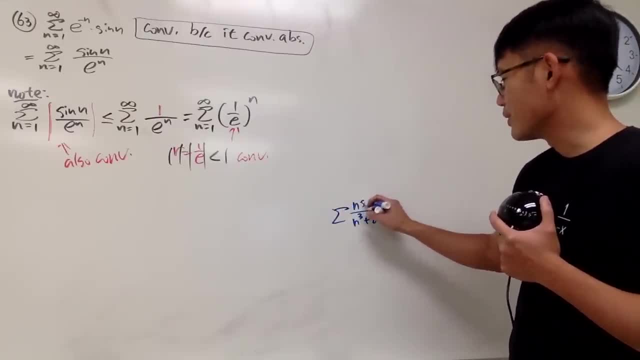 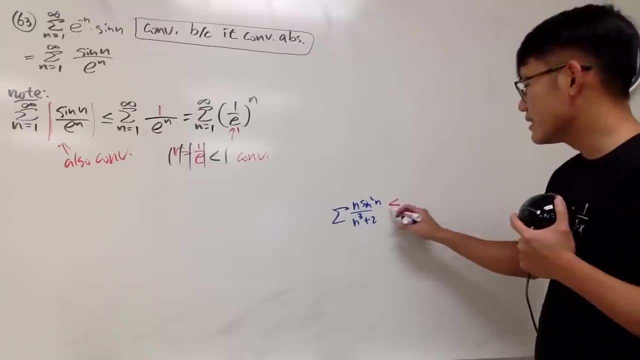 I don't remember how long ago, This right here, right Plus 2 or so, sine squared n, like this: Technically I should not put the absolute value, Technically I should just say less than or equal to n times 1, like this: 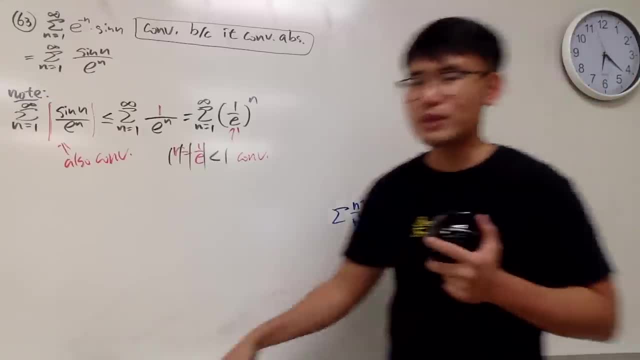 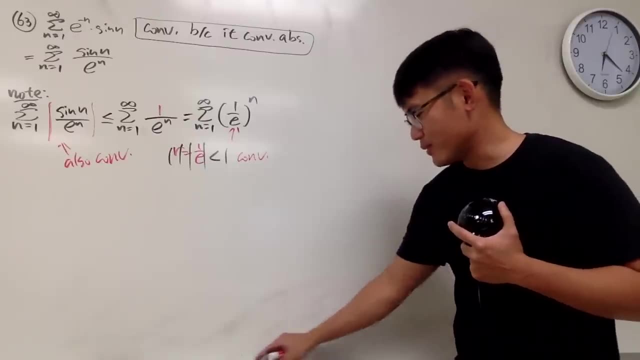 I should not put the absolute value, because it was all well, but everything was positive, so it was okay. so All right. It gets kind of tricky if you want to talk about some proofs, if you want to talk about some rigorous proofs. 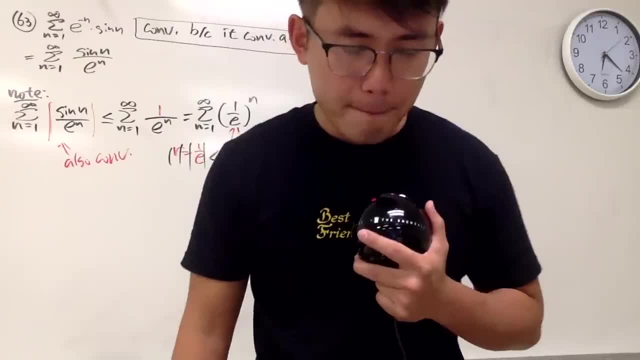 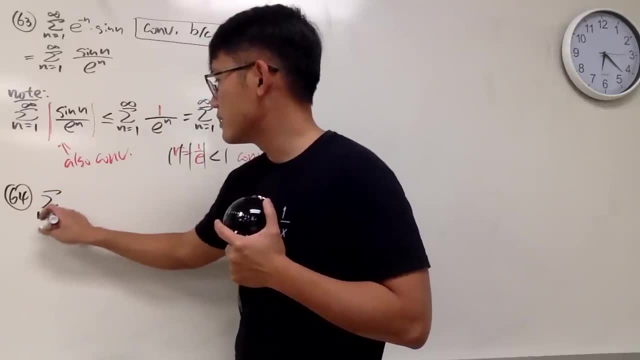 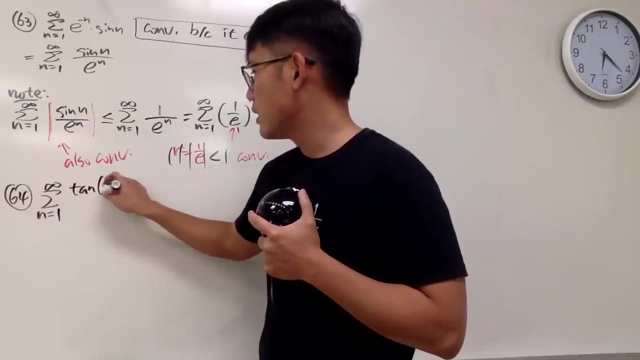 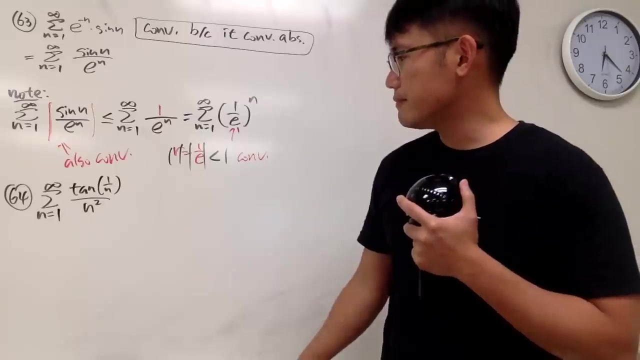 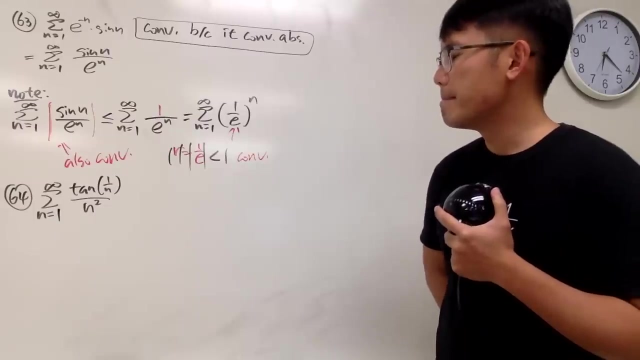 By the way, number 63, done, Number 64.. Sum as n goes from 1 to infinity Time squared like this, Hmm, Well, well, Maybe comparison test works, huh, Because it's like something over 1 over. 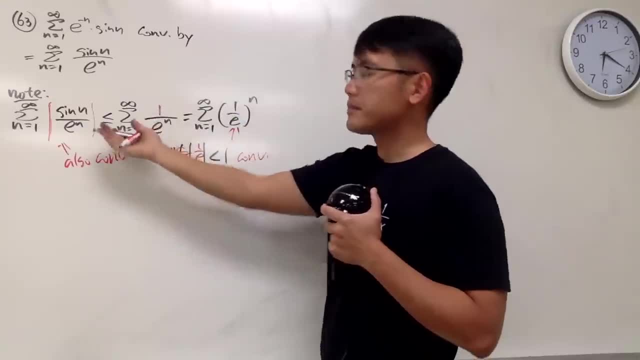 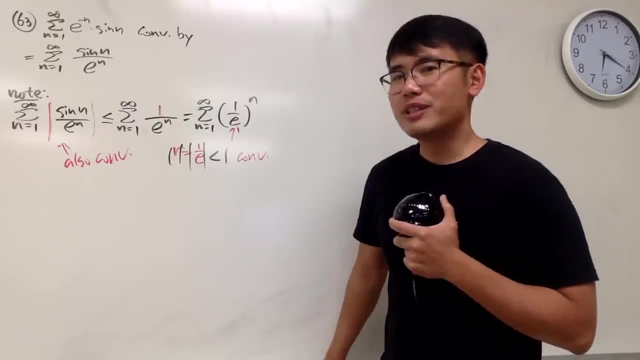 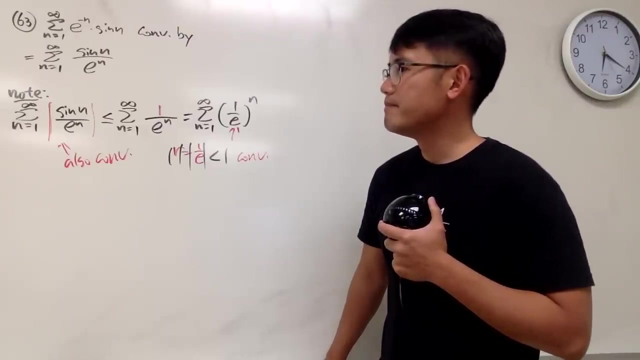 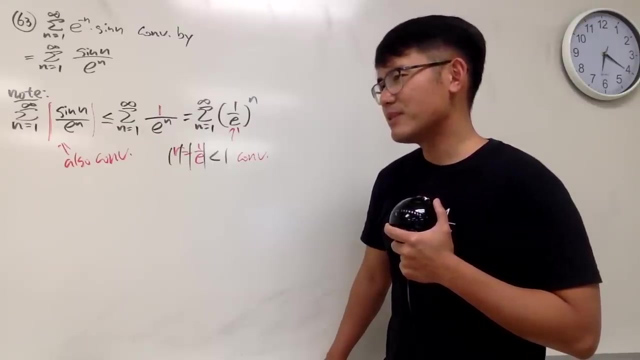 It converges as well, and it's actually by comparison test. I will actually say, hmm, ah yeah, this is kind of tricky, because for comparison test I should have said, oh yeah, that's tricky. Oh man, when I take the absolute value for the cosine 1.. 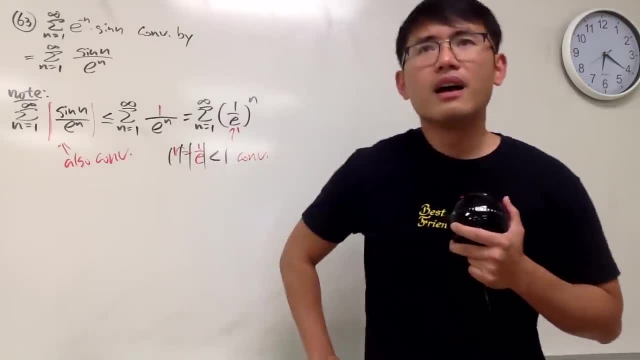 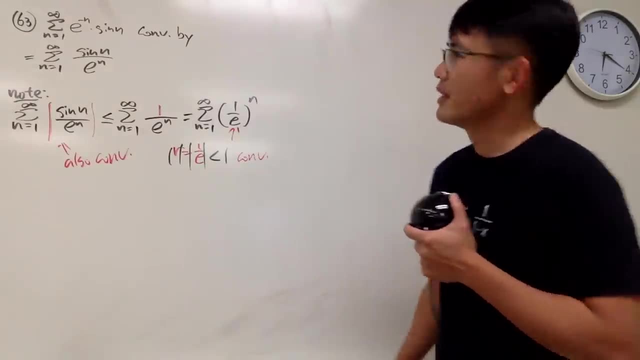 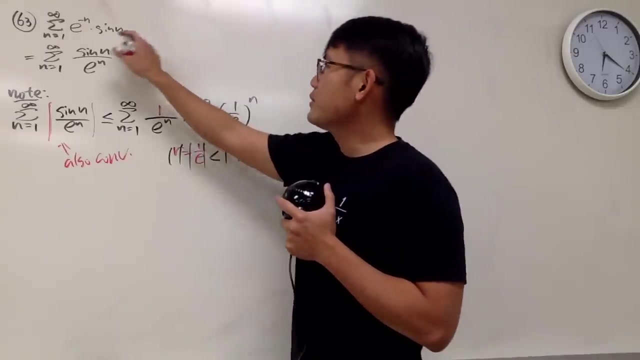 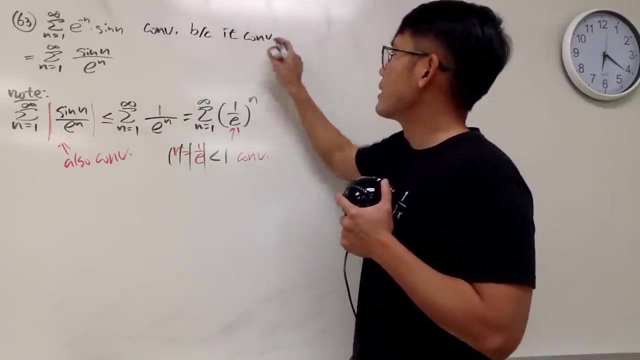 Oh no, that was The alternating, so I was good. Okay, didn't make that mistake earlier. Okay, so here is the deal. This is why that this actually converges, okay, This right here converges because it converges absolutely. 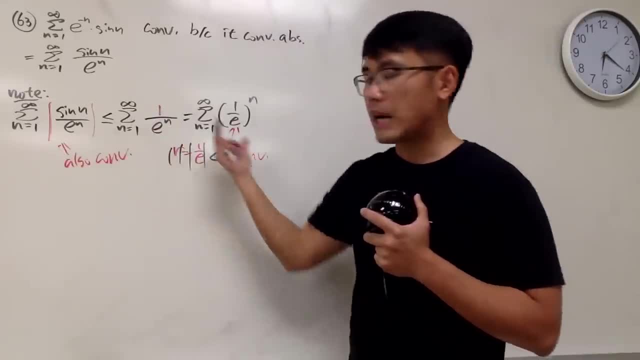 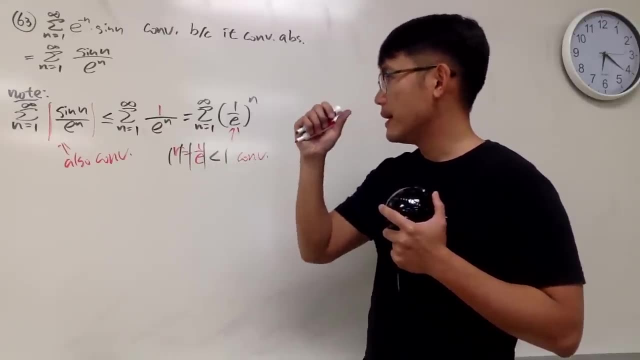 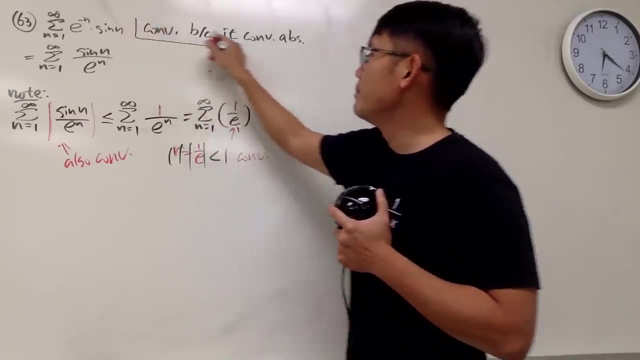 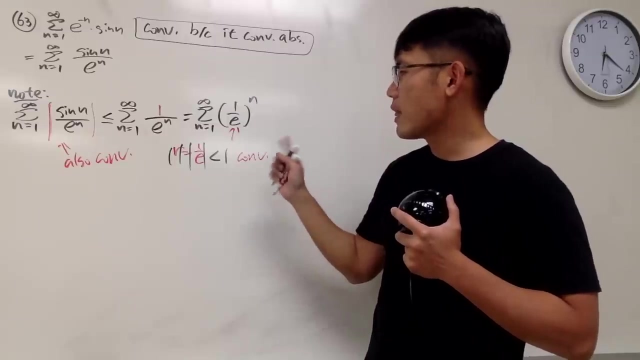 Why? Because the absolute version right here, based on the comparison test, it works. Right, based on the comparison test, it works and, yeah, converges absolutely. because it converges absolutely. and the absolute value version, this right here, is the when, this, when everything is positive, you can do the comparison test. 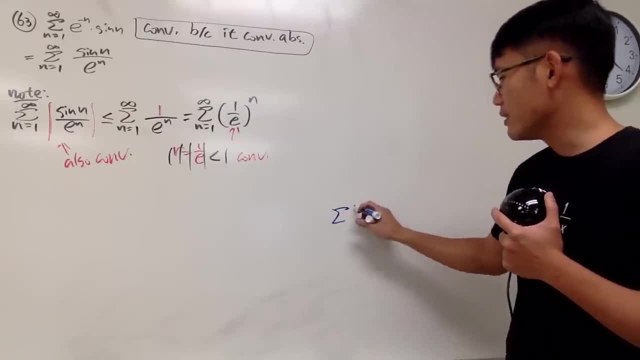 So that kind of reminds me of the question that we did like earlier- I don't remember how long ago- This right here, right plus 2 or so, sine squared n, like this: Technically I should not put the absolute value. 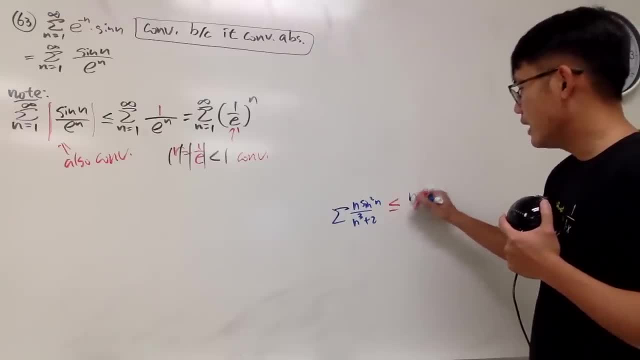 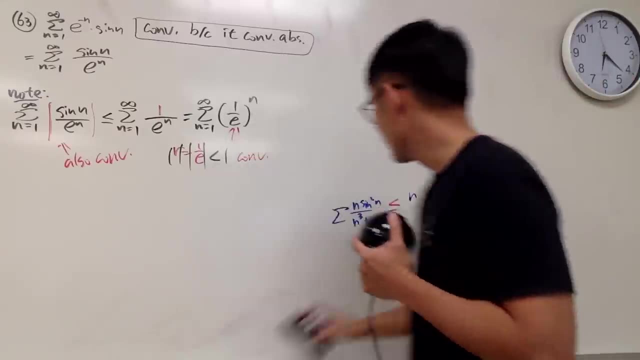 Technically, I should just say less than or equal to n times 1, like this. I should not put the absolute value because it was all Oh, but everything was positive, so it was okay. so All right. it gets kind of tricky if you want to talk about some proofs. 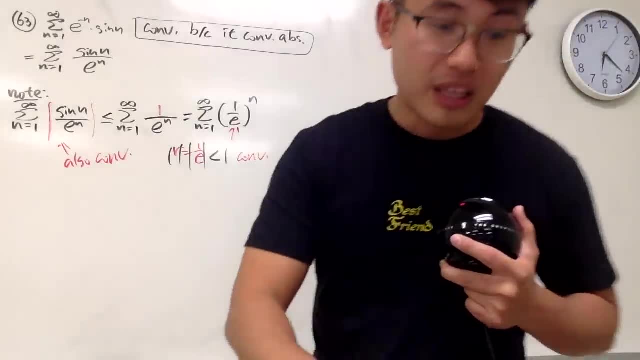 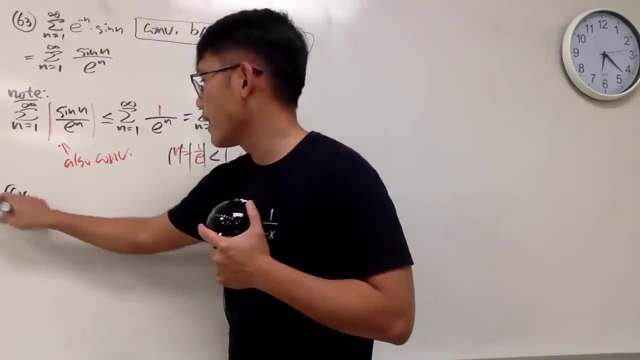 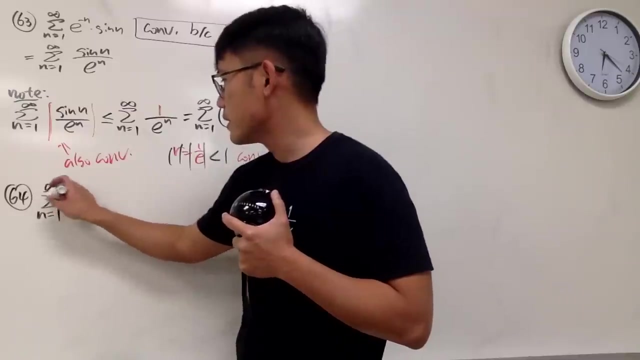 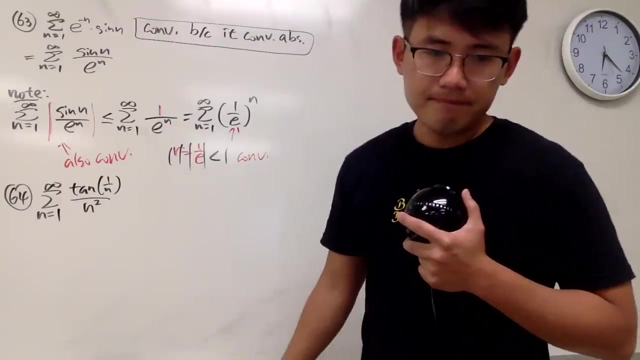 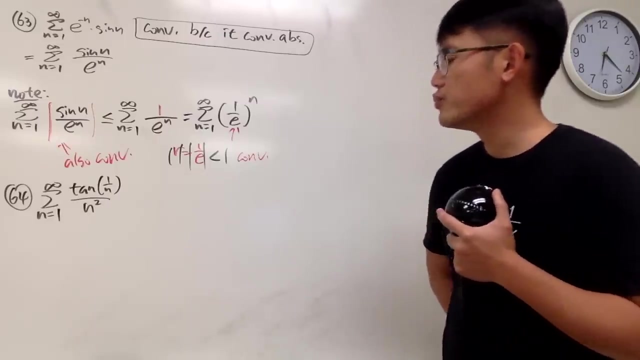 You want to talk about some rigorous proofs, But anyway, number 63, done. Number 64, sum as n goes from 1 to infinity, n squared like this: Hmm, Well, well, Maybe comparison test works, huh. 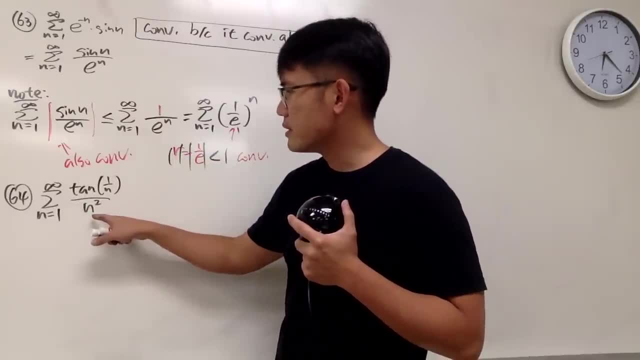 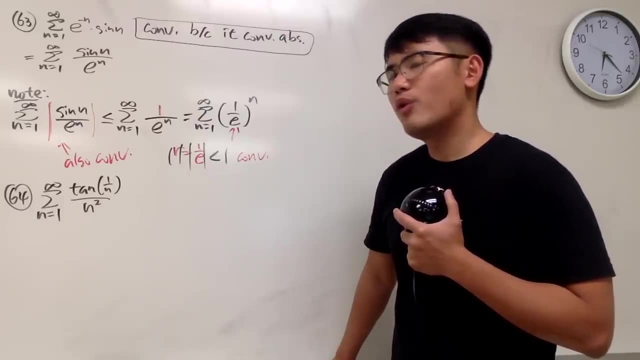 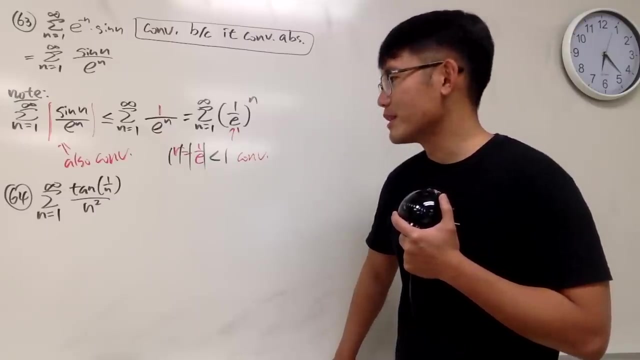 Because it's like something over 1 over Hmm, Tangent 1 over n. If tangent 1, tangent of 1, is tangent of 1 radians, Hmm, No, I don't know how big that is. 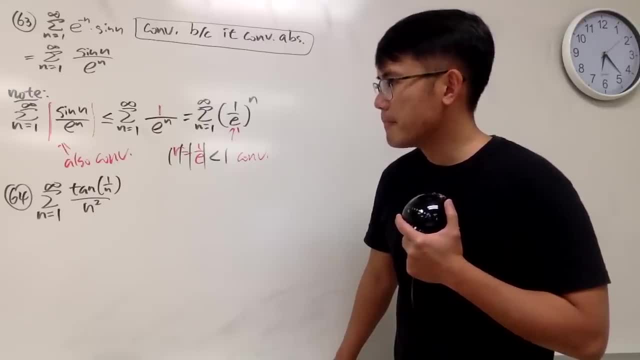 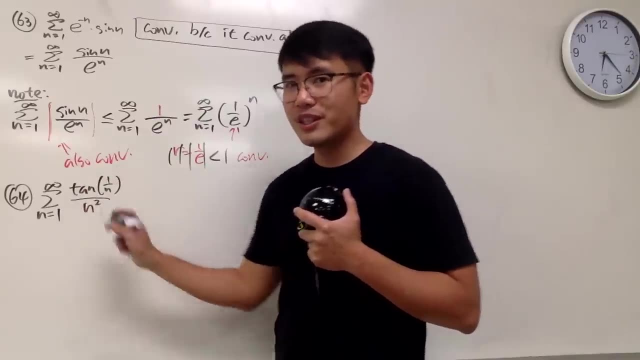 Oh man. Hmm, I was going to just do the integral. I think I'm just doing the integral test, Why not? If you check seriously, you can really check this right here On the top. well, I'll just write this down right here. 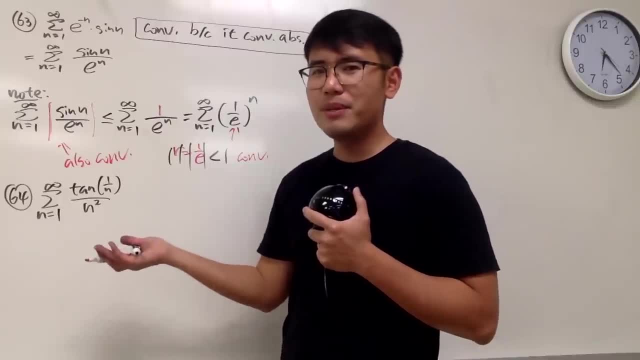 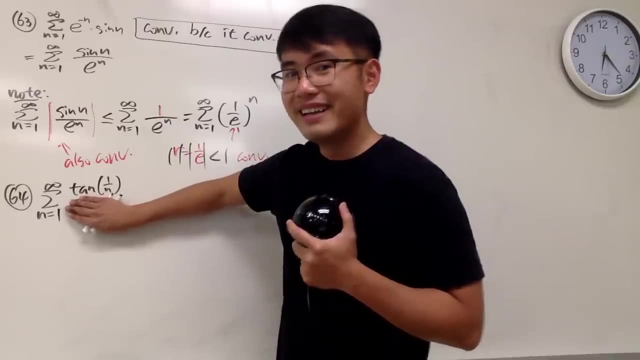 Let's do the integral test. If you want to do the direct comparison test, maybe, But not the limit comparison test with 1 over n squared. If you do that, you end up with this part only, And then that will give you 0, so that's not good. 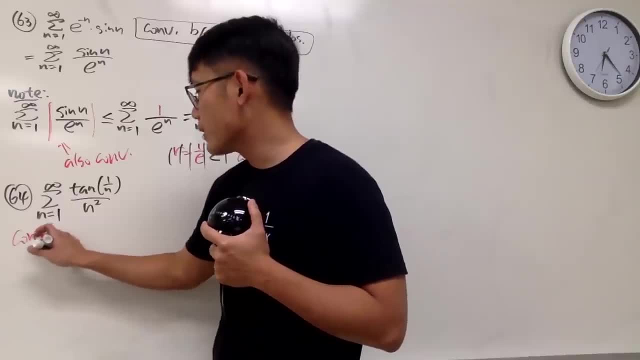 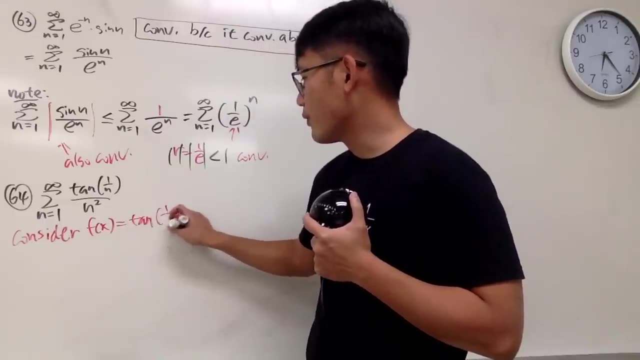 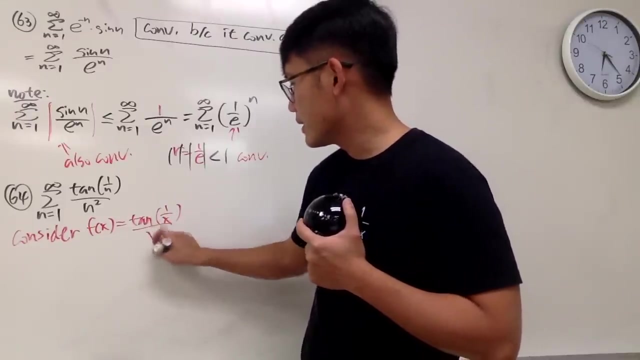 But anyway, I'll just do the integral test. So I will just Tell you guys to consider f of x being tangent of 1 over x over x squared. Yeah, Like this, Okay, So consider that and let's do some integral real quick. 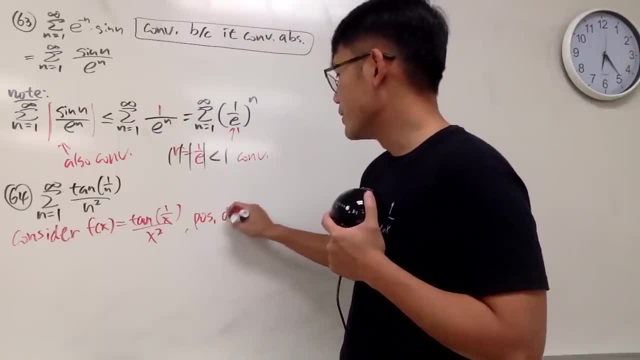 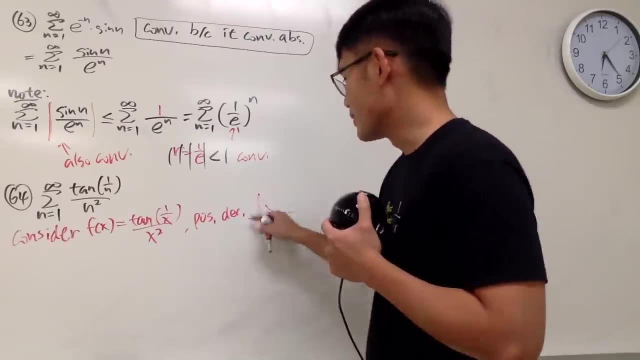 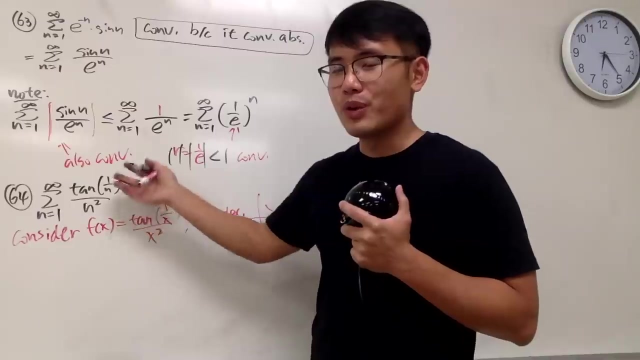 And, of course, just go ahead and say positive decreasing And seriously show a graph first before you say that, okay, Let's Much more legitimate than just Just show. Anyway, here we go. If you want to use a graph, you can also show: this is less than or equal to 1 over x squared. 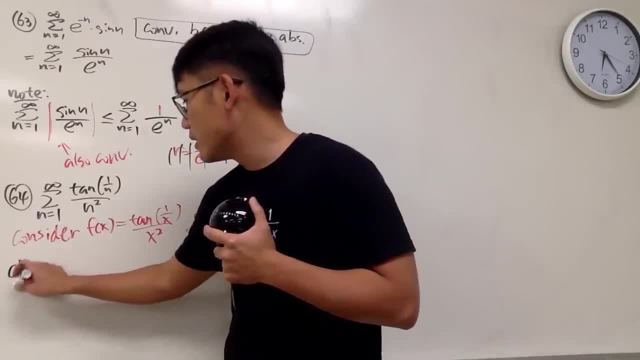 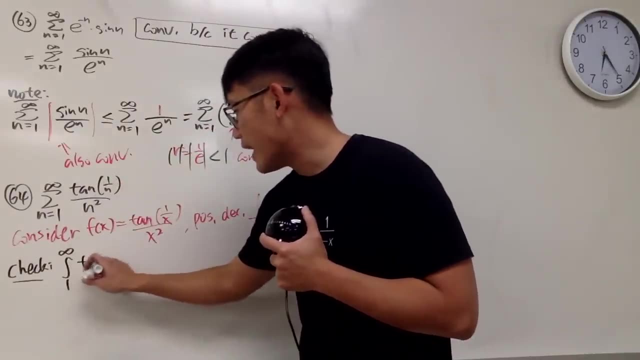 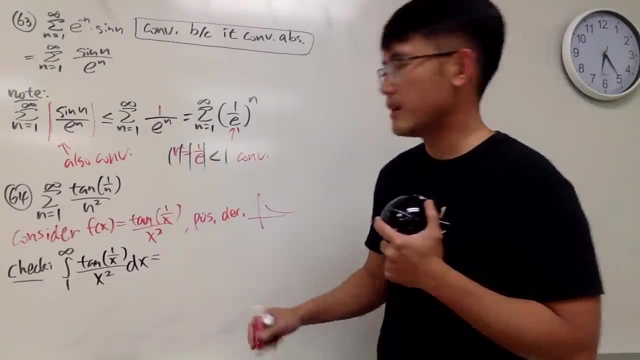 But like, let's do integral real quick, It's not that bad at all. So check the integral, Improper integral from 1 to infinity. Here we have tangent 1 over x over x squared dx. Now let's do this in our head, all right. 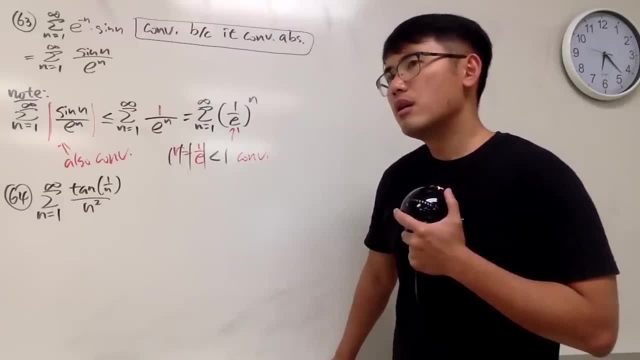 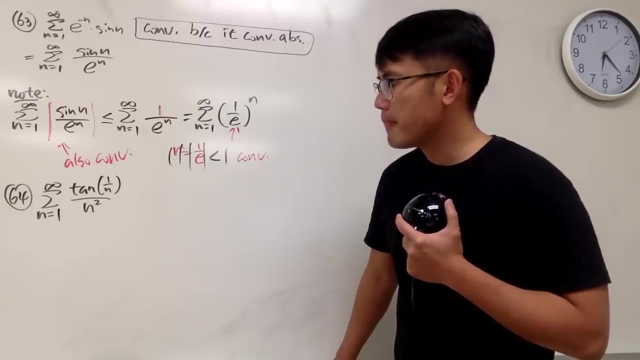 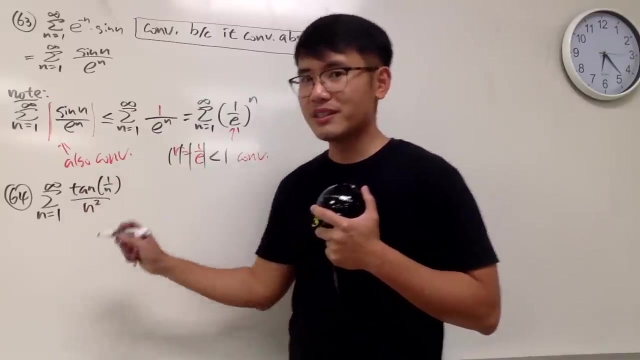 Hmm, Tangent 1 over, and if tangent 1, tangent of 1, is tangent of 1 radians? hmm, no, I don't know how big that is, man, I was going to just do the integral. I think I'll just do integral test, why not? if you check seriously, you can really check this right here on the top. well, I'll just write this down right here. let's do the integral test. 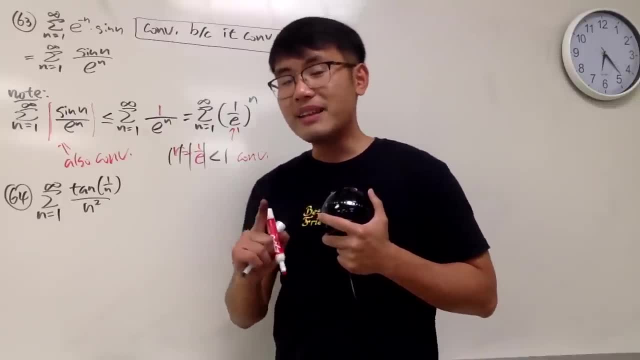 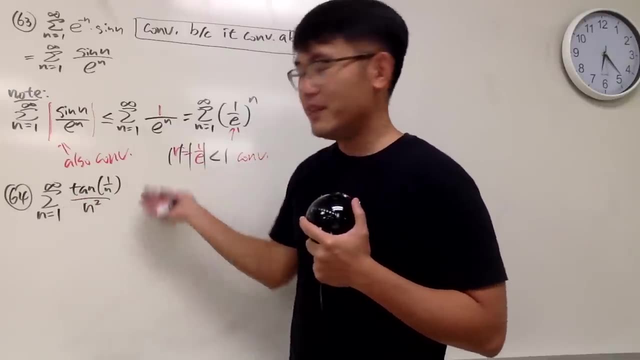 if you want to do the direct comparison test, maybe, but not the limit comparison test with 1 over n squared. if you do that, you end up with this part only, and then that will give you 0, so that's not good. 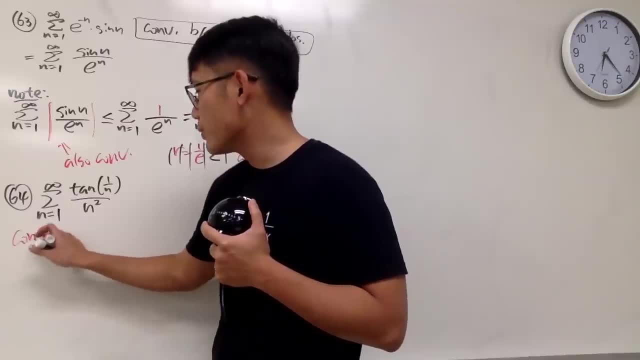 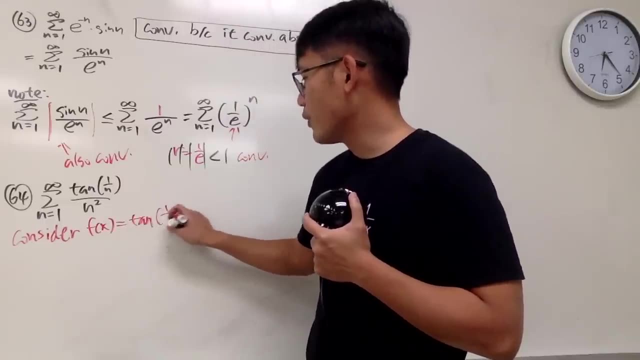 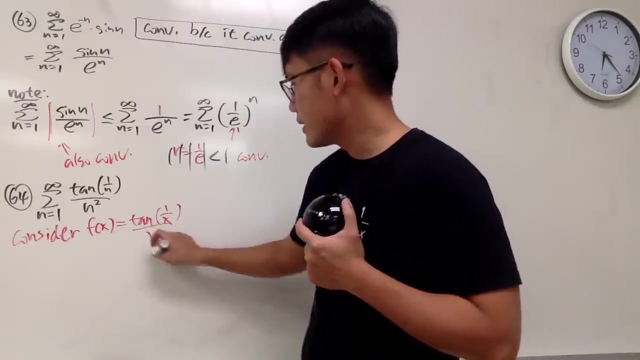 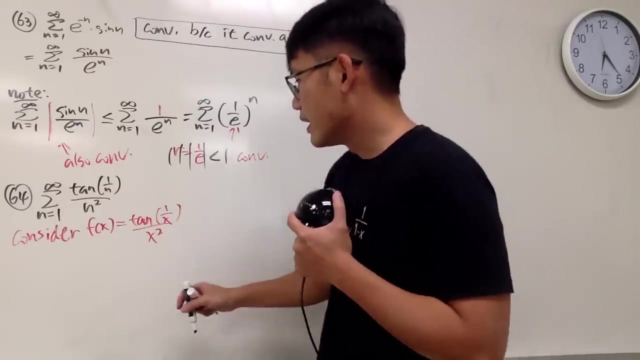 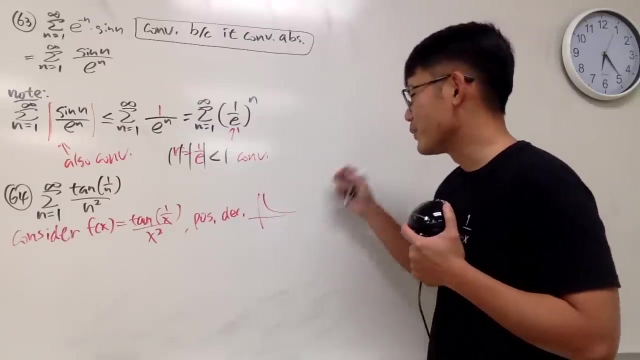 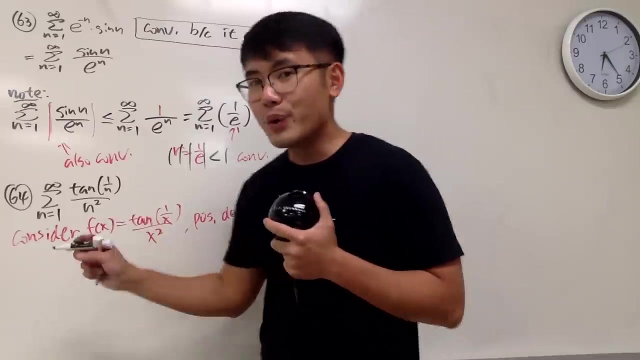 finally, I'll just do the integral test. so I will just tell you guys to consider f of x being tangent of 1 over x over x squared. yeah, like this. okay, so consider that and let's do some integral real quick. and, of course, just go ahead and say positive decreasing and seriously show a graph first before you say that, okay, that's much more legitimate rather than just just just show anyway, here we go. if you want to use a graph, you can also show: this is less than or equal to 1 over x squared. but, like, let's do integral real quick, it's not that bad at all. 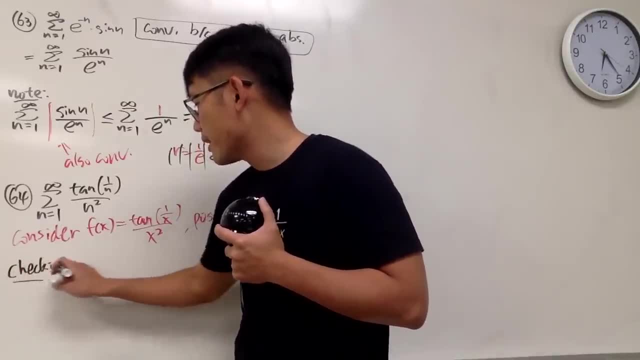 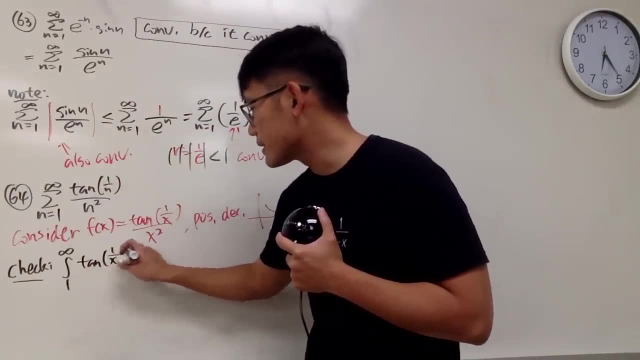 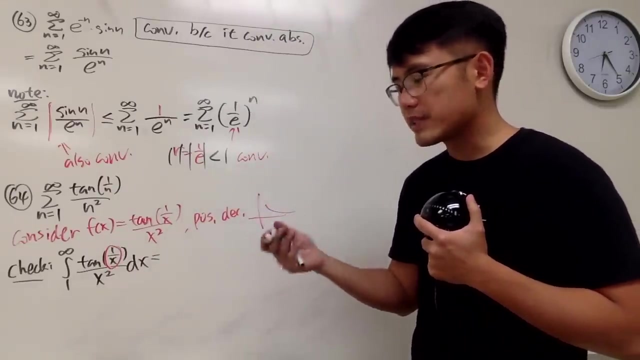 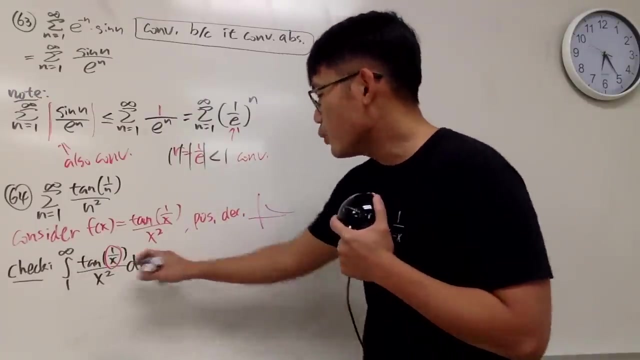 so check the integral integral, improper integral from 1 to infinity. here we have tangent 1 over x over x squared dx. now let's do this in our head, alright, so you take u to be 1 over x and if you differentiate that you get negative 1 over x squared. so the idea is that you should have a negative sign right here so you can get that right. so the integral for that is 1 over x squared. 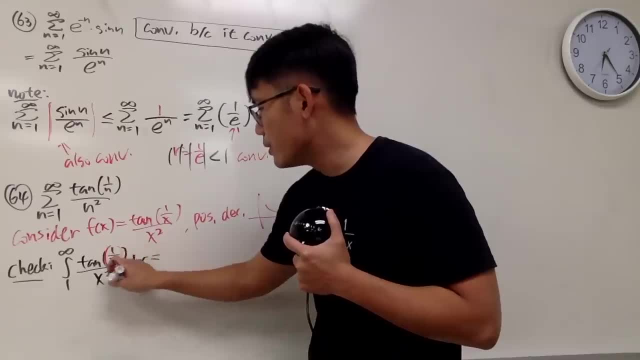 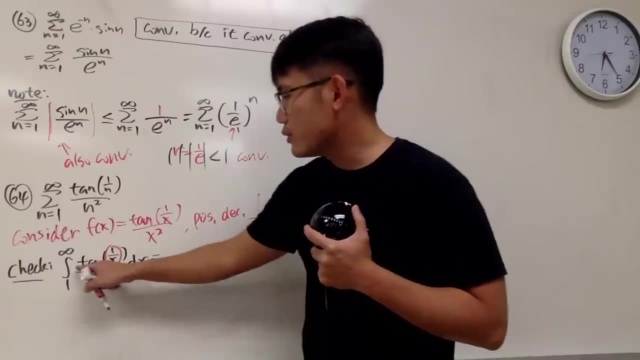 So you take u to be 1 over x And if you differentiate that you get negative 1 over x squared. So the idea is that you should have a negative sign right here So you can get that right. So the integral for that is going to be: 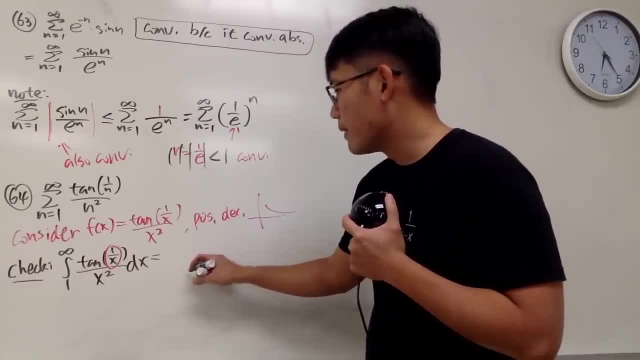 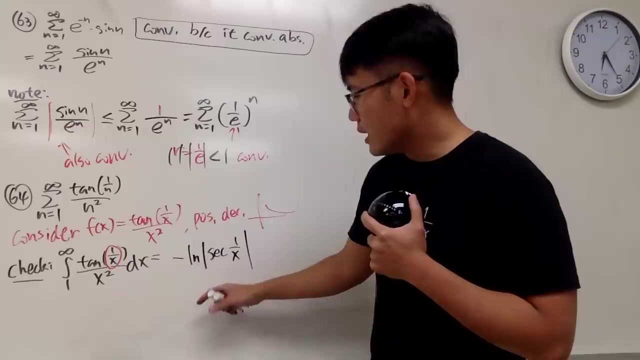 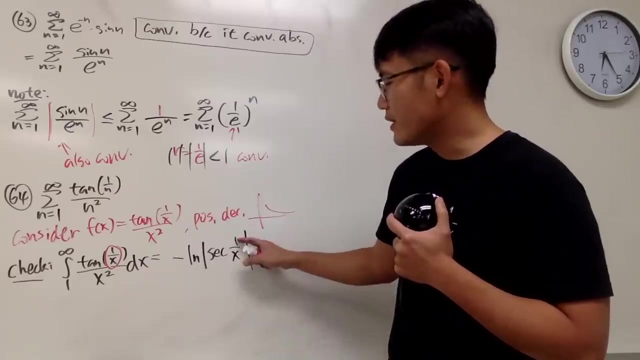 so you get negative: 1 over x squared. now let's see what's going to be. okay, let's alright. let's do everything in our head: natural log, absolute value, secant of 1 over x, like this: and what's the negative in the front? why? because if you have natural log of secant u, that will give you tangent right. but you have to differentiate this. you get negative, which will cancel, you get positive and you end up with 1 over x squared. 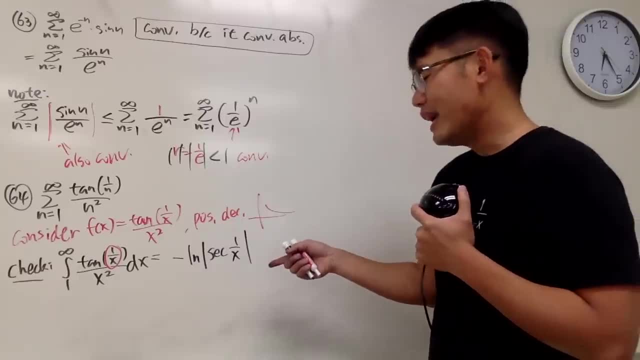 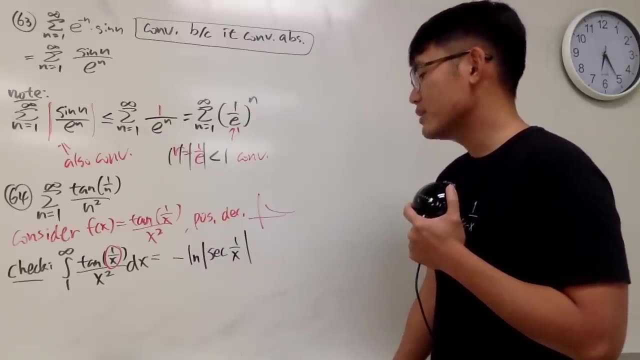 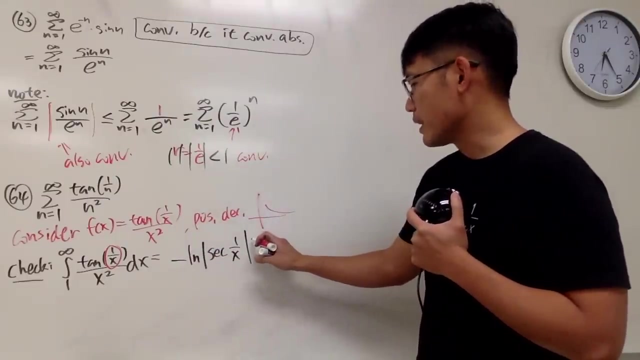 x squared, so this right here is legitimate, and in that case you can actually write this down as cosine. so, uh, that's a good idea. so perhaps let's just do it like that. actually, let's just keep it like this. anyway, here we go and we just plug in, plug in, so we get going from one to infinity. 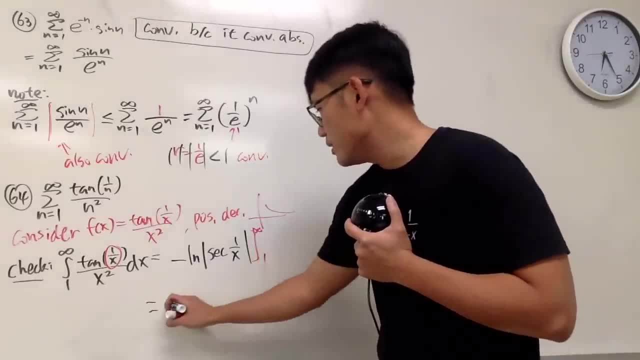 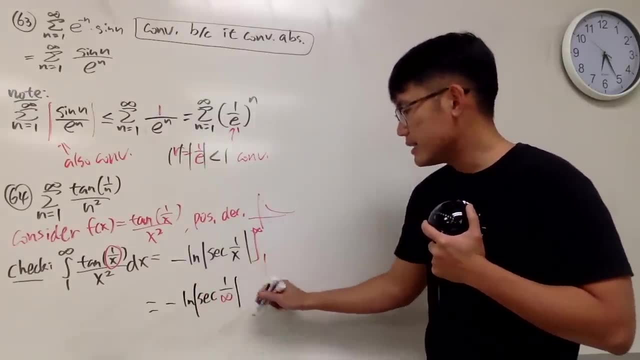 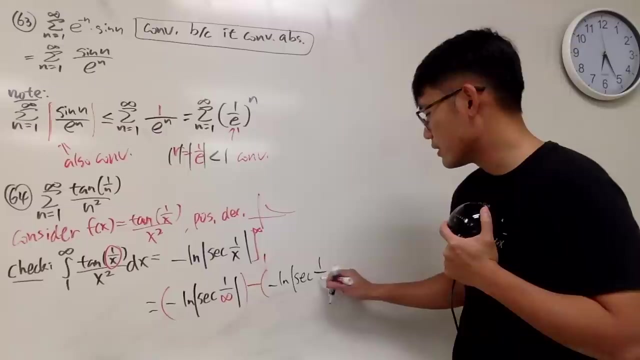 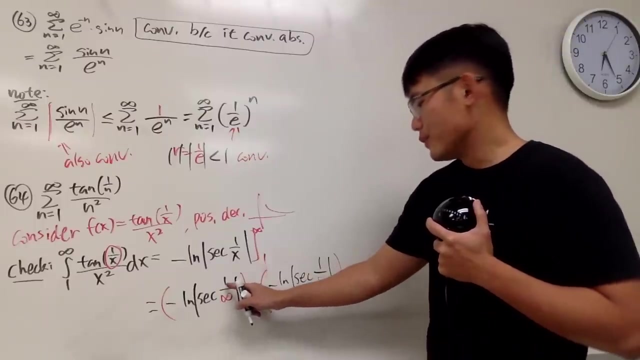 so this is going to be negative ln absolute value, secant of one over infinity and minus, minus, negative ln absolute value secant of one over zero, like this right. so now, secant of- well, this is actually well, come on, it's not one, it's not zero, it's one. 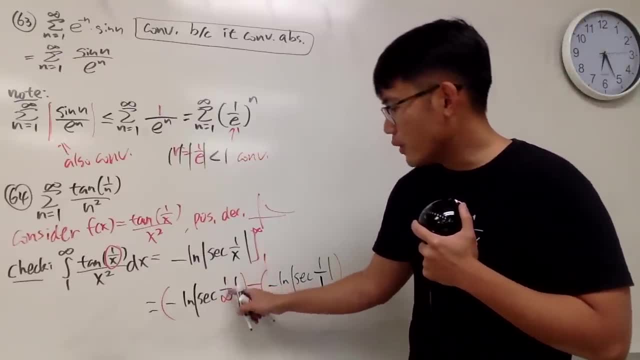 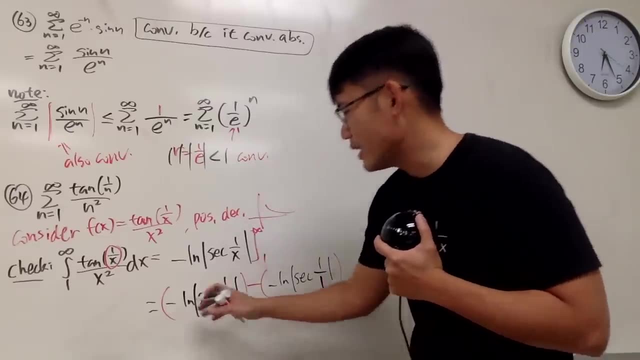 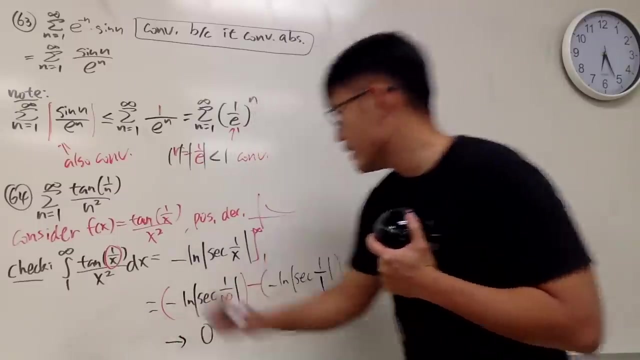 okay, this one here is a triple sum, because one over infinity is zero, but luckily, secant of zero is just one. so the whole thing right here is just l and one. in another way it's just zero. and actually i have to draw arrows now because we're taking the limit and right here 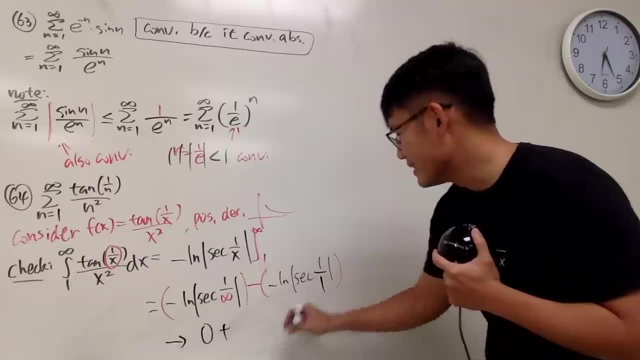 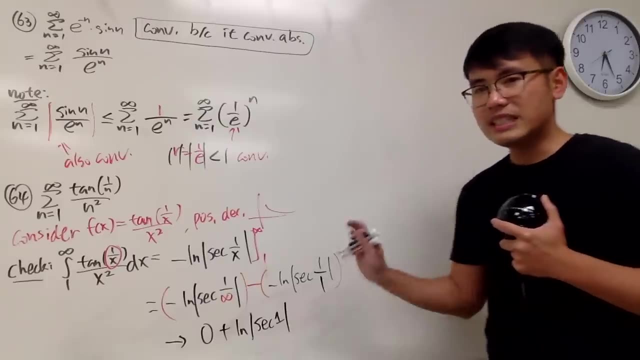 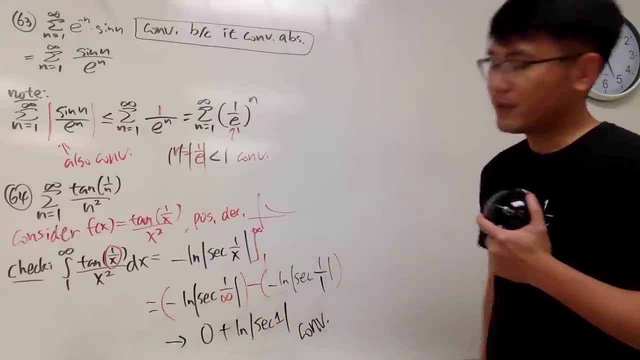 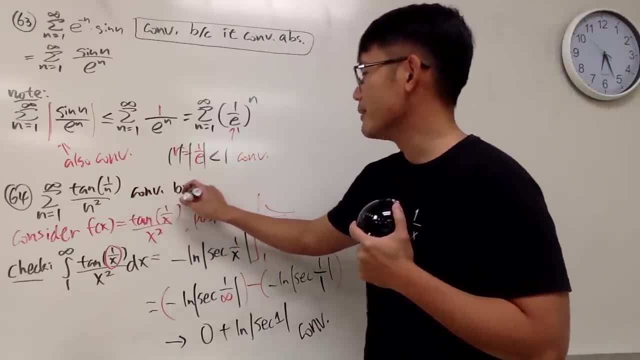 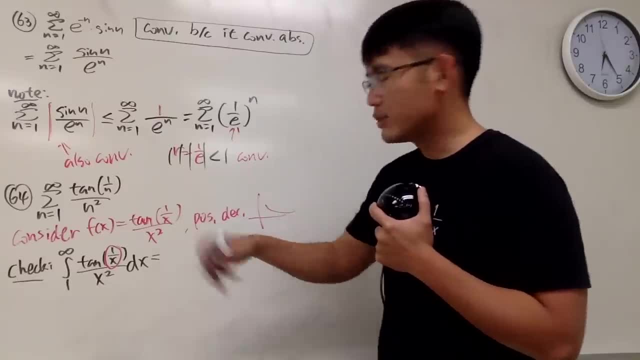 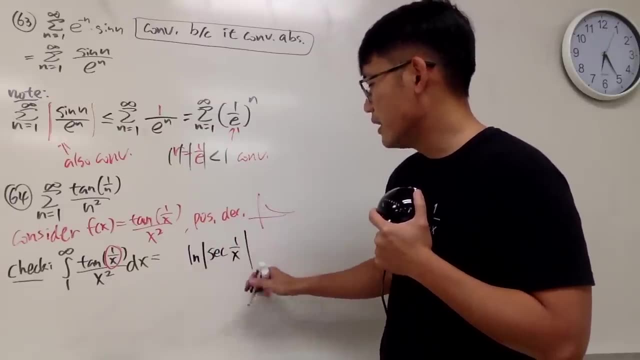 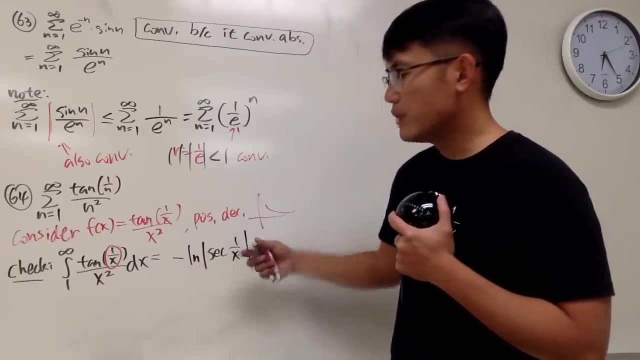 Okay, Let's All right, let's do everything in our head. Natural log- absolute value secant of 1 over x. Like this: And what's a negative In the front? Why? Because if you have natural log of secant u, that will give you tangent right. 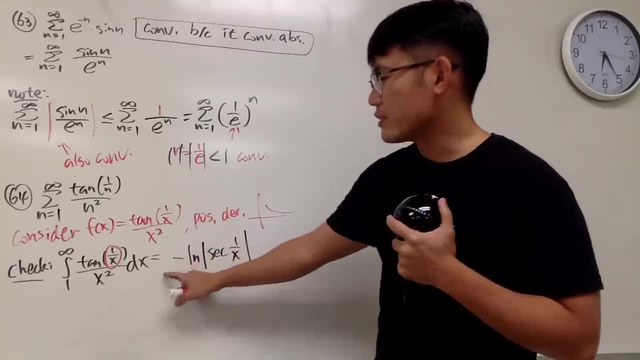 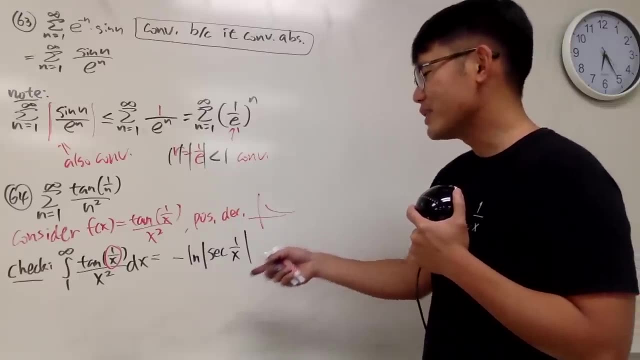 But you have to differentiate this. You get negative, which will cancel. You get positive And you end up with 1 over x squared. So this right here is legitimate, And in that case you can actually write this down as cosine. 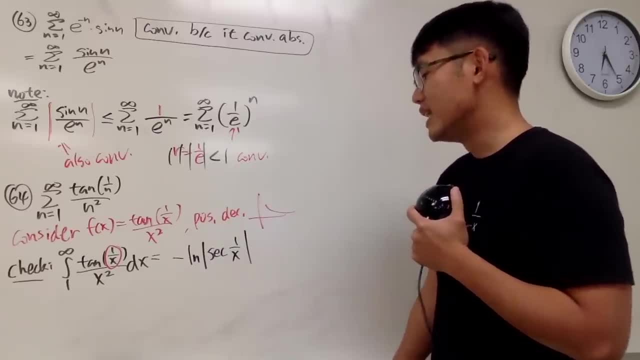 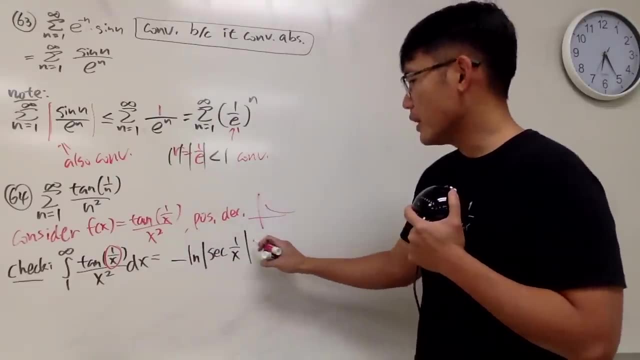 So that's a good idea. So perhaps let's just do it like that. Actually, let's just keep it like this. Anyway, Here we go, And then we just plug in, plug in, So we get going from 1 to infinity. 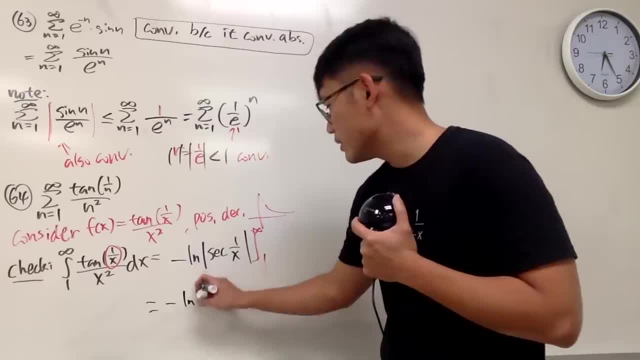 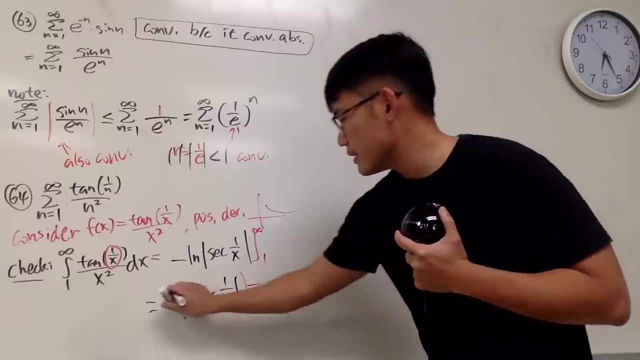 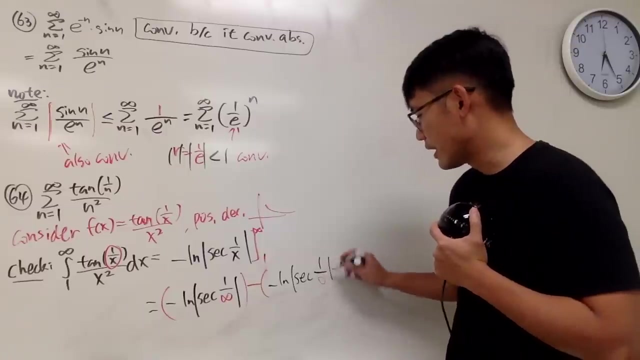 So this is going to be negative ln absolute value secant of 1 over infinity, And minus negative ln absolute value secant of 1 over 0.. Like this Right. So now, secant of, Secant of. Well, this is actually. 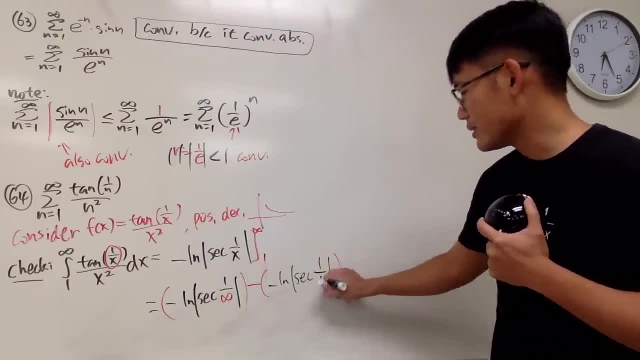 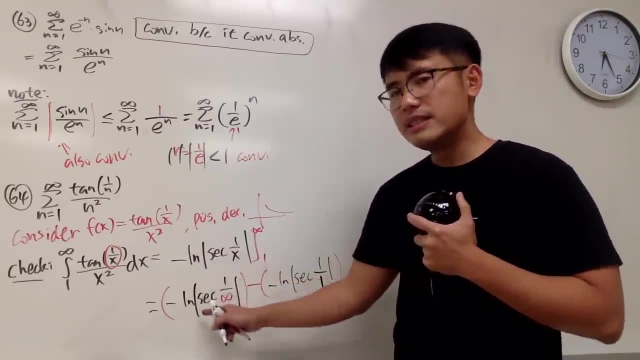 Come on, It's not 1.. It's not 0. It's 1.. Okay, This right here is a triple sum, Because 1 over infinity is 0. But luckily, secant of 0 is just 1.. 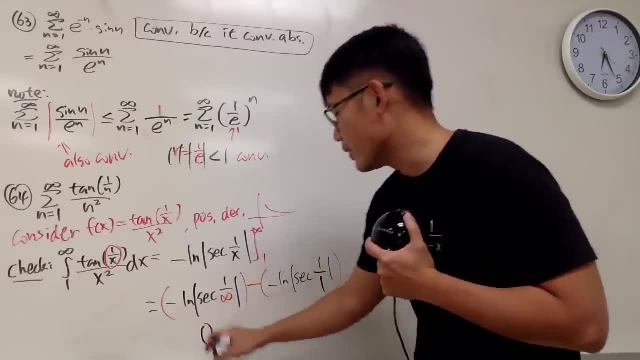 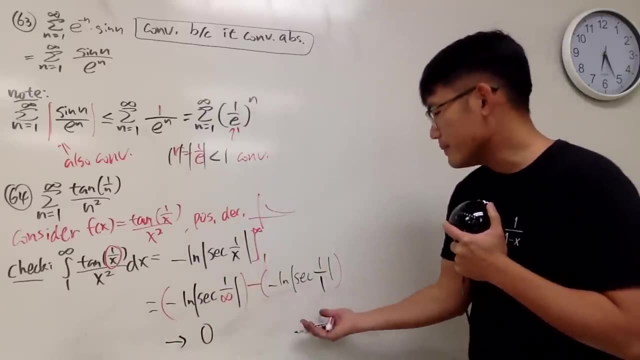 So the whole thing right here is just ln 1.. In another words, just 0.. And actually I have to draw arrows now because we're taking the limit And right here, negative, That's positive And this is natural log. 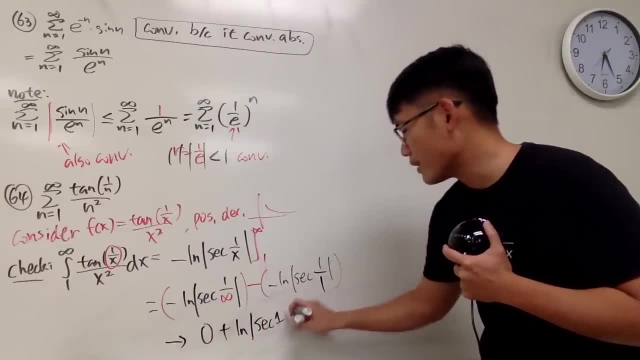 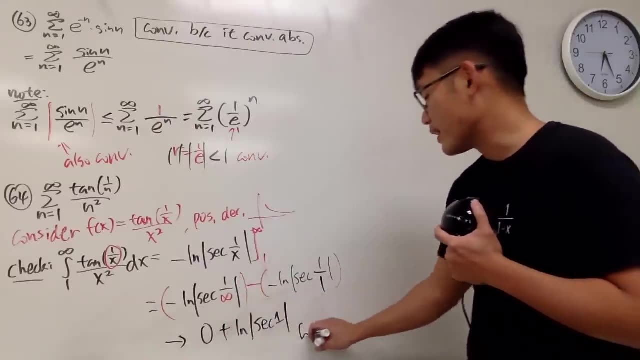 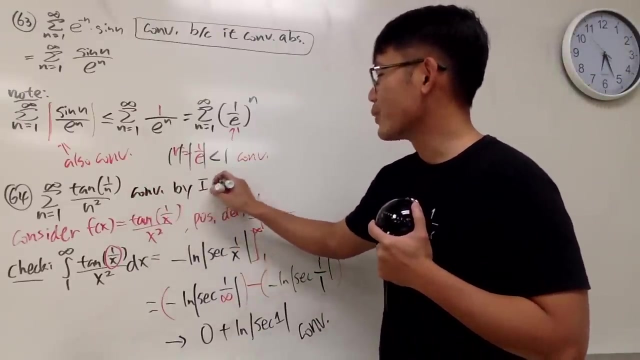 Absolute value And we have secant of 1.. This is the safe number because it's not secant of pi over 2 whatsoever right. So this right here, finite, Therefore converges. If this converges, this right here also converges by the integral test. 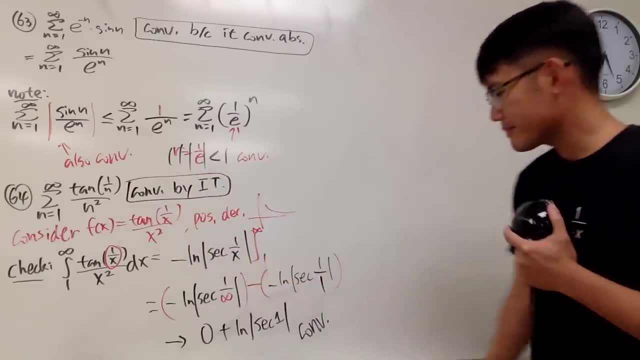 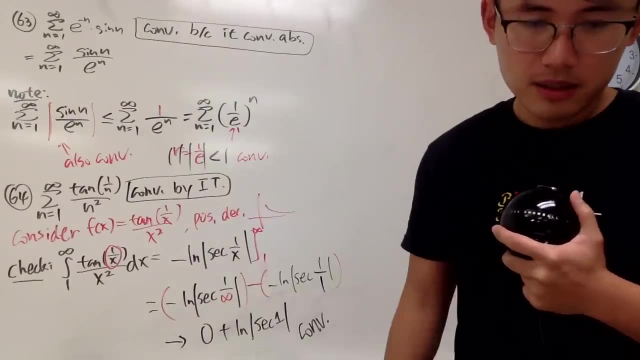 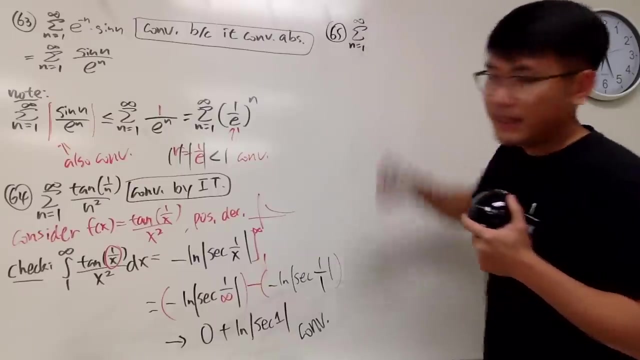 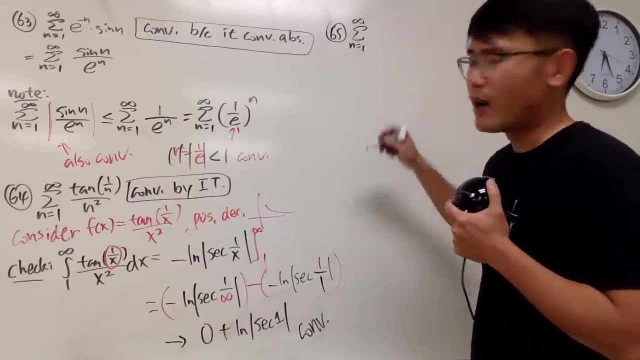 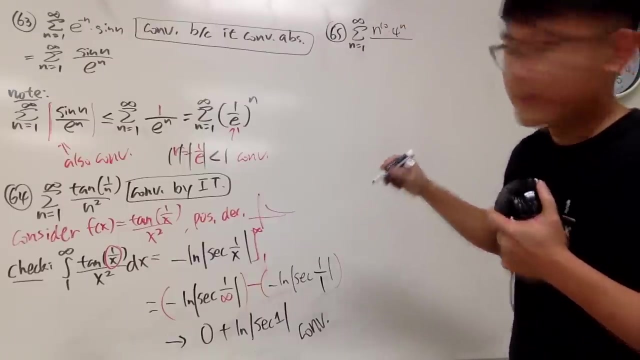 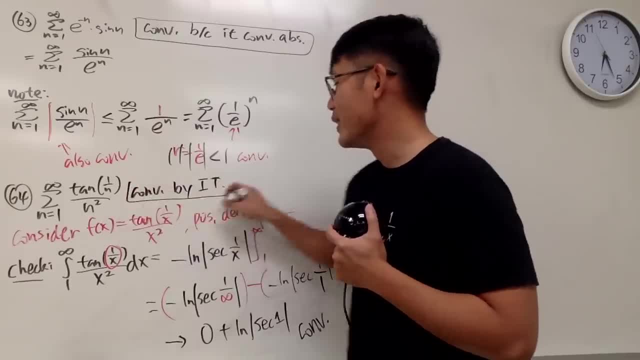 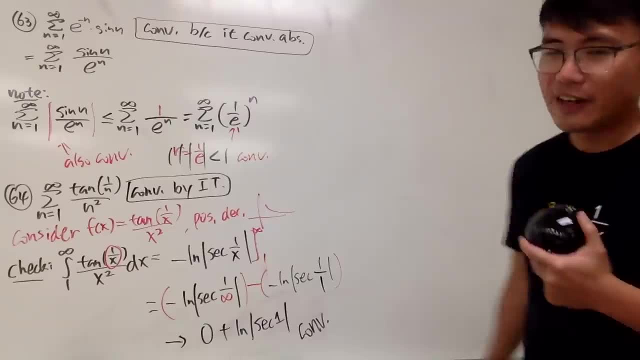 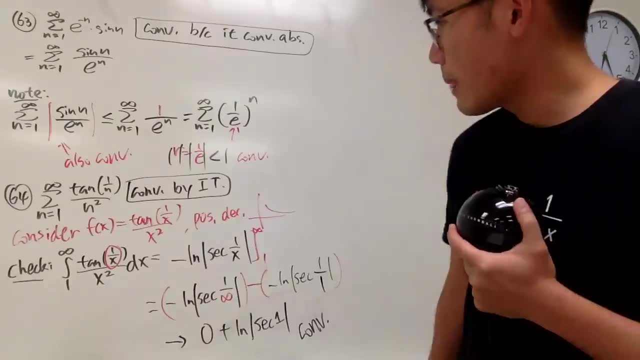 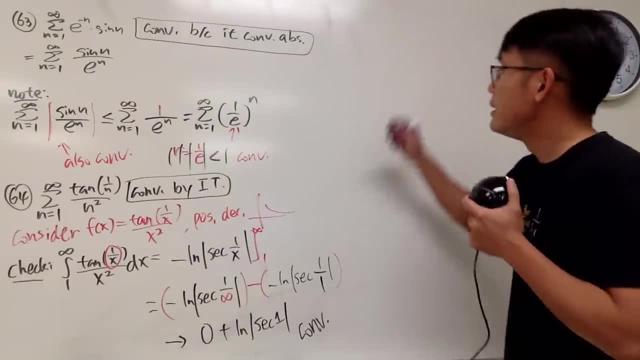 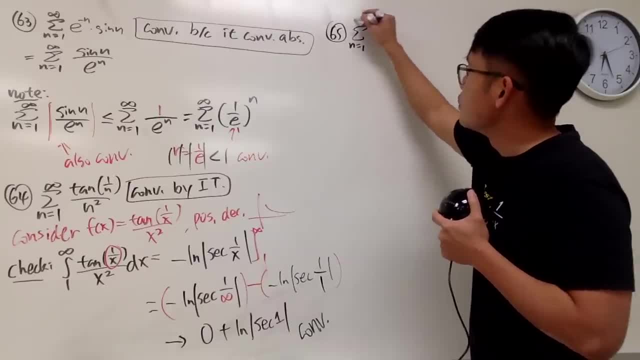 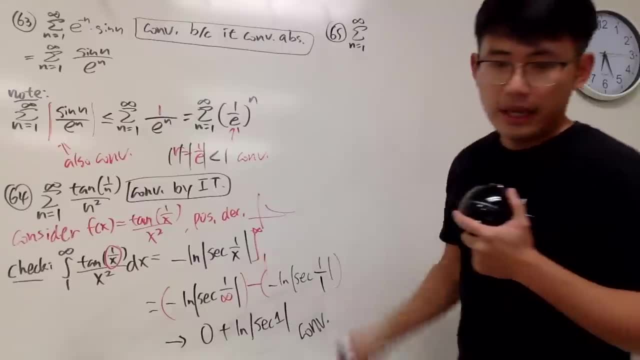 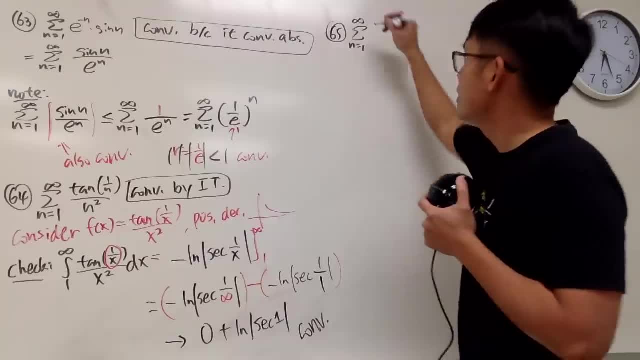 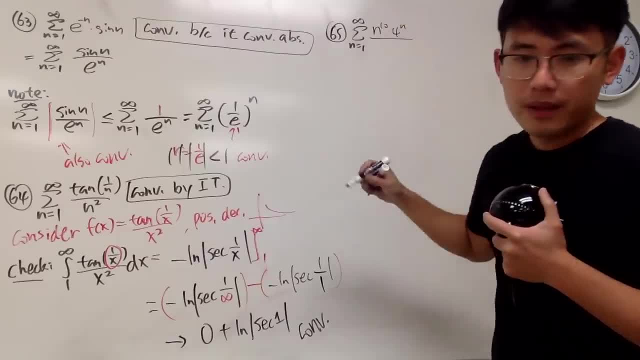 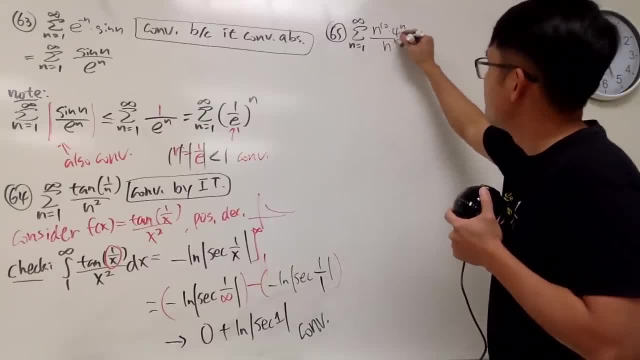 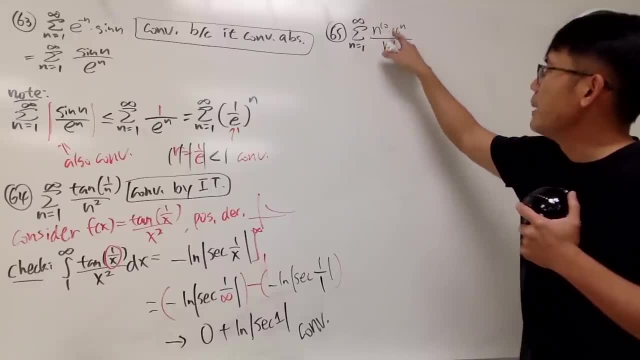 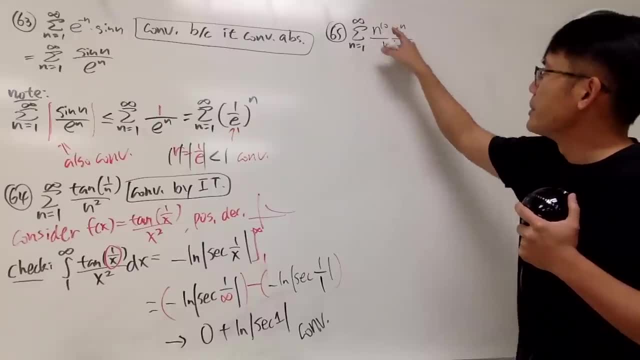 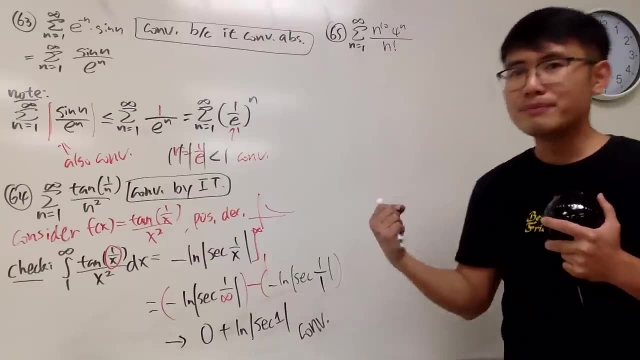 Interesting Because you know n to the p and b to the n. they are both smaller than n factorial. But today, if they decide to team up by multiplying, I don't know if they will be the n- factorial or not. 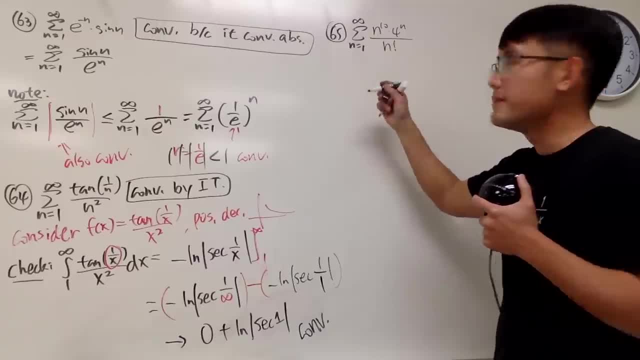 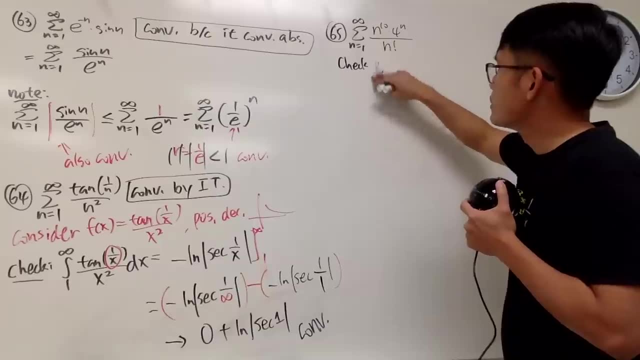 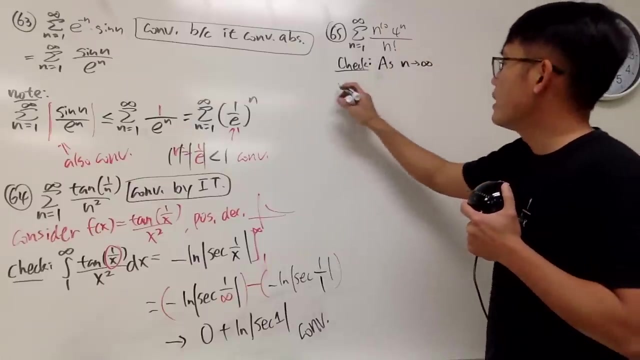 We'll see. So, anyway, let's do a ratio test. Yeah, So here we go. I'll just say: check As n goes to infinity. Well, this right here. we are just going to look at the absolute value again. 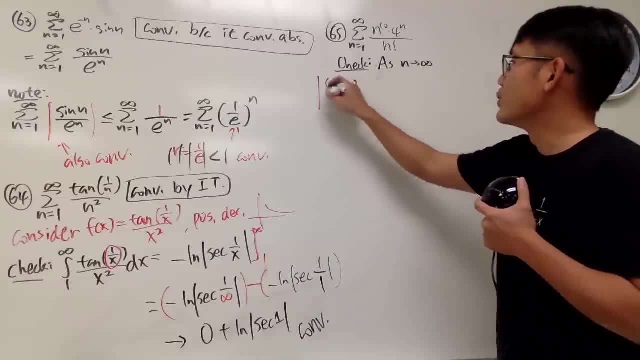 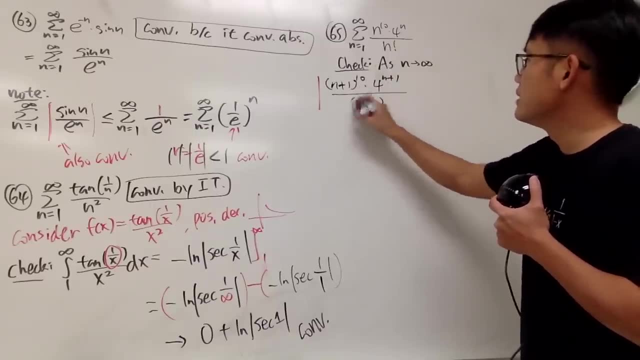 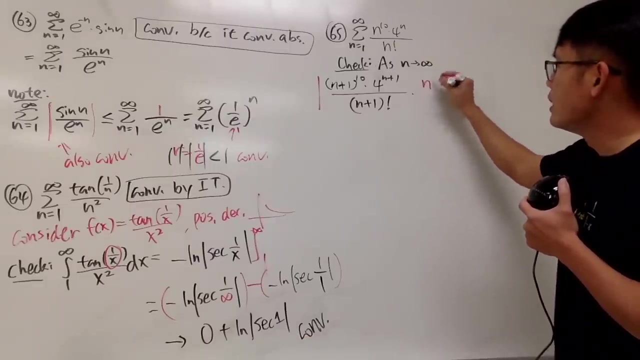 Okay, And here we have. We have n plus 1 to the 10th power, multiplying with 4 to the n plus 1, divided by n plus 1 factorial. And for the other part, right here we have just the reciprocal of the original. 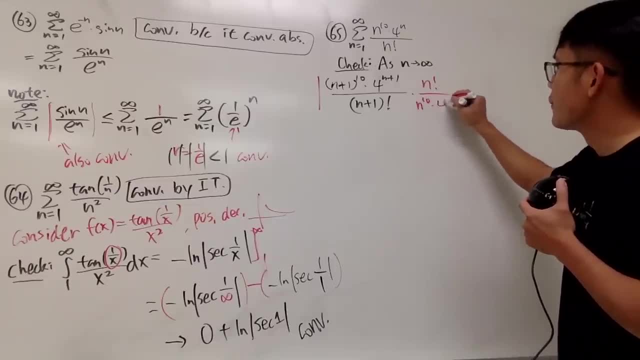 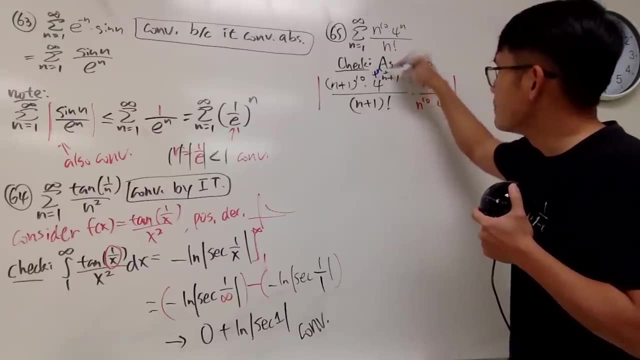 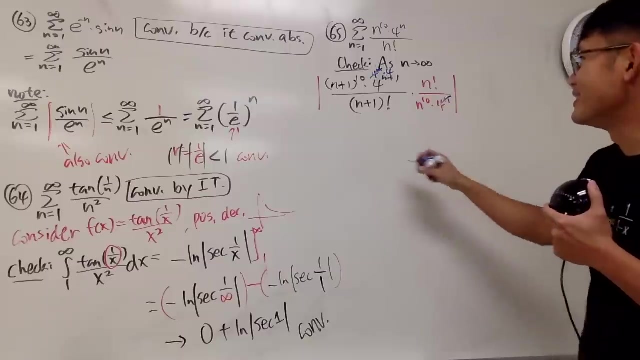 n, factorial over n to the 10 times 4 to the n, like this. Now, here is the deal, This right here is 4n times 4.. So that's not too bad. And cancel, cancel, already Seriously right. 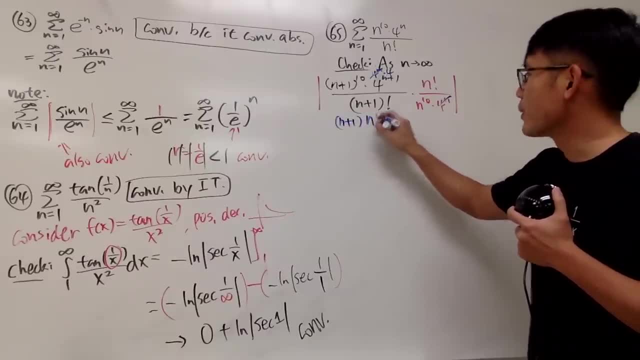 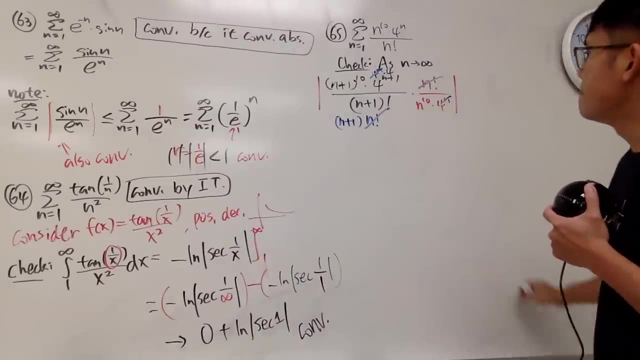 And this right here is n plus 1 times n factorial. So this and that will be out right away, And that's also very nice. Hmm, What else do we need to do? Okay, So again this and that: cancel out the 4.. 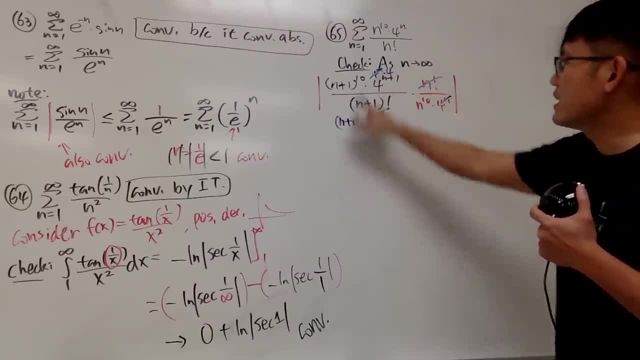 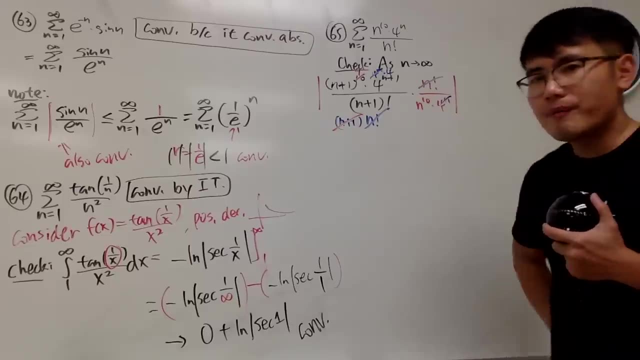 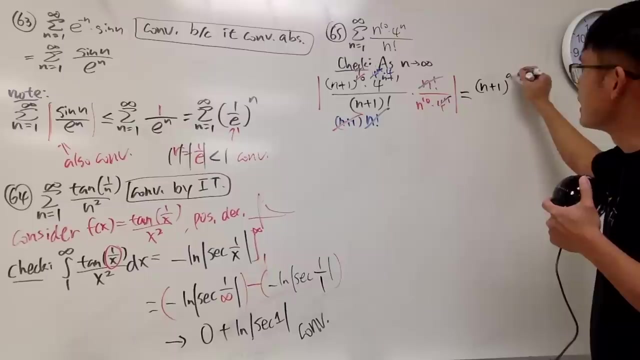 So it's right there, But This, and that we can reduce that a little bit, So let's cancel this. And this is 9, right? So that's all the simplifications that we will have, And on the top now it's just n plus 1 raised to the 9th power. 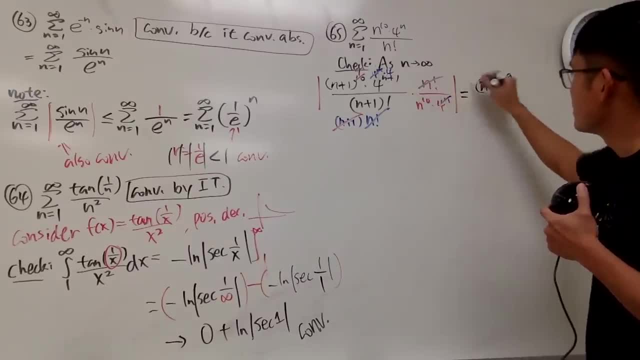 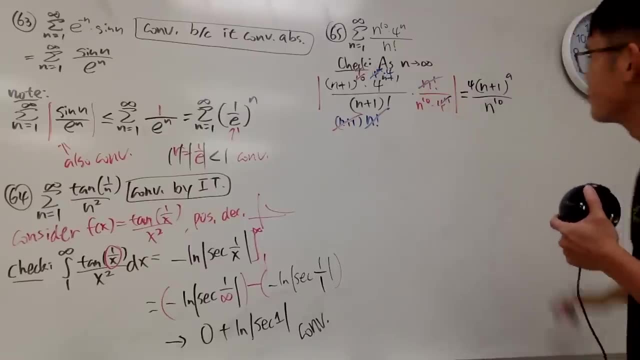 And then on the Well also to multiply by the 4, but it's not a big deal, But I still want to put that down. And on the bottom we have n to the 10th power, This right here: power function over power sequence. power sequence right. 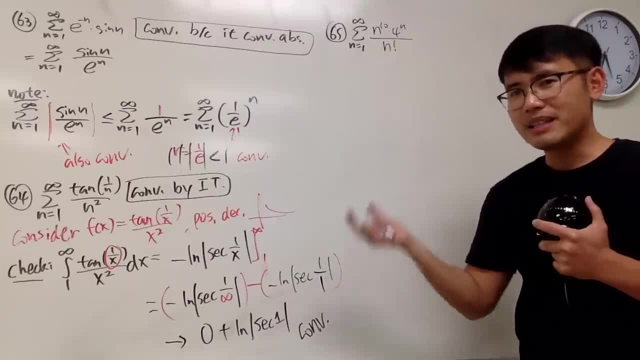 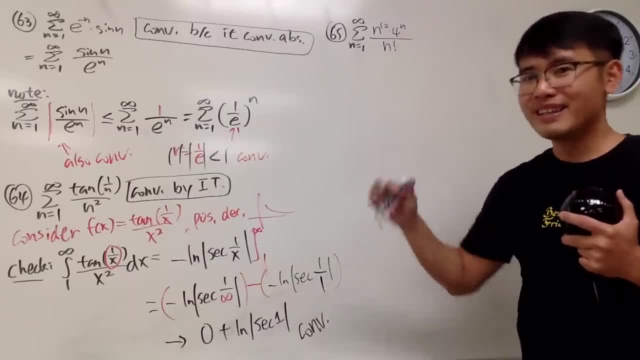 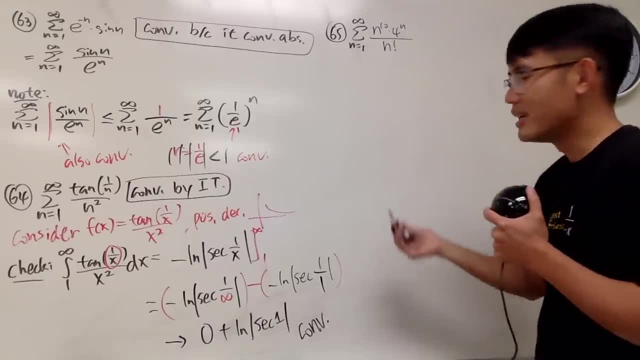 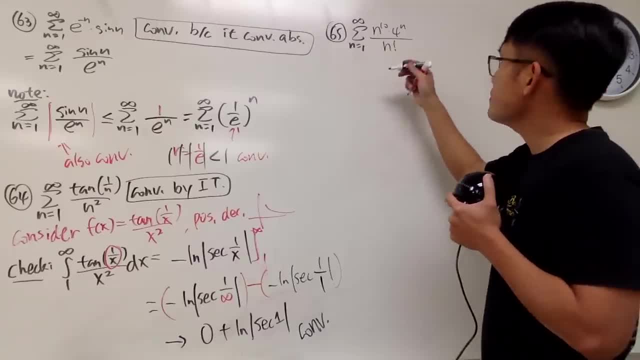 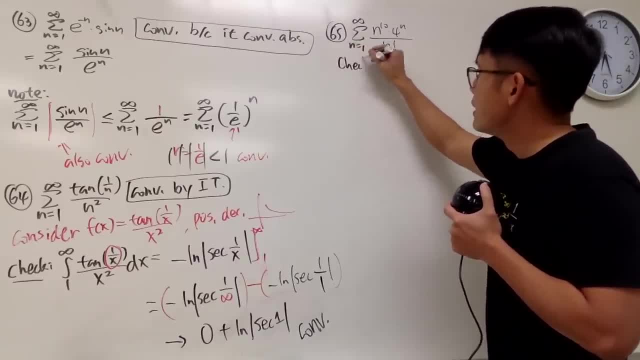 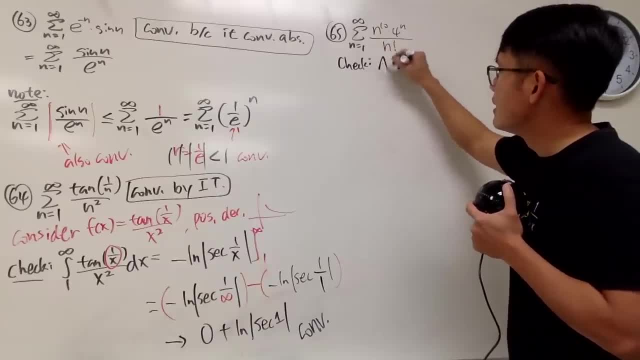 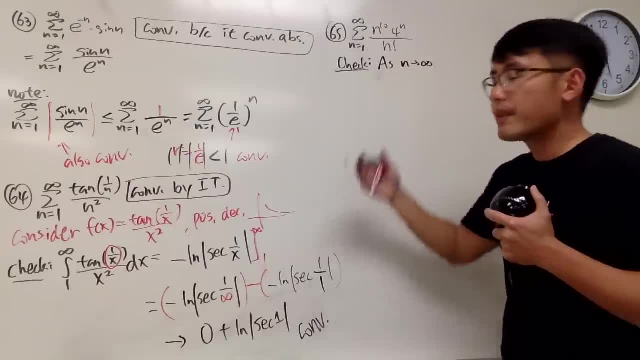 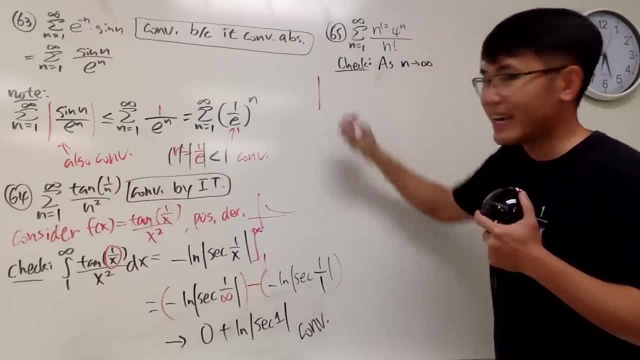 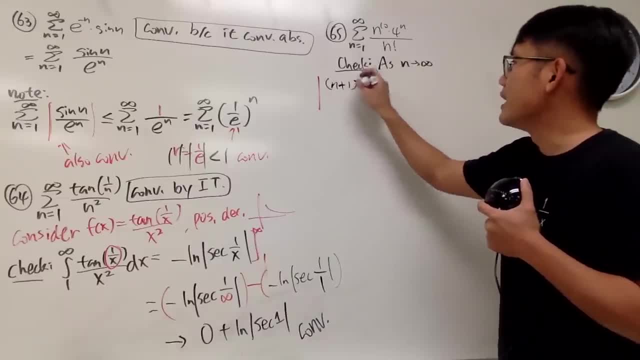 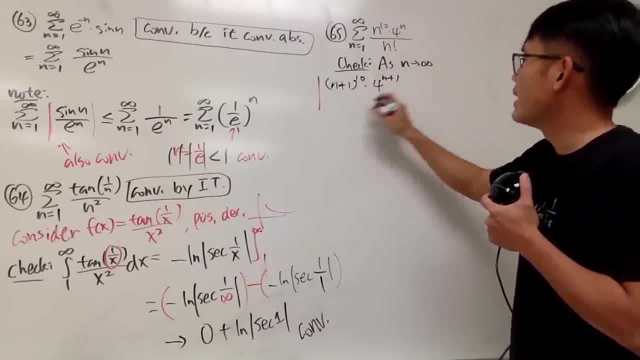 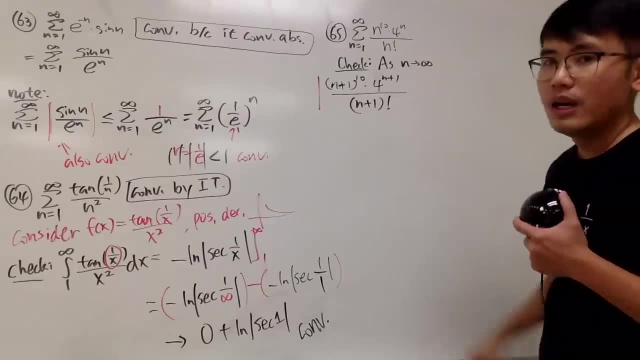 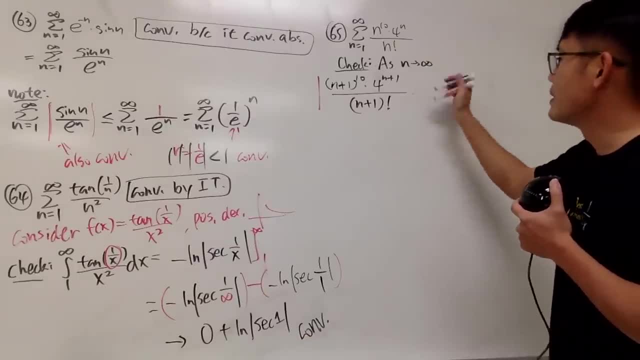 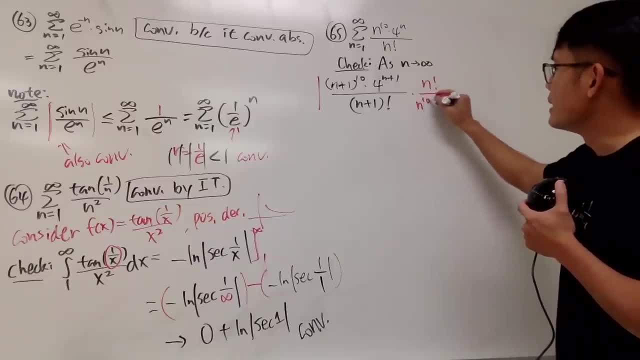 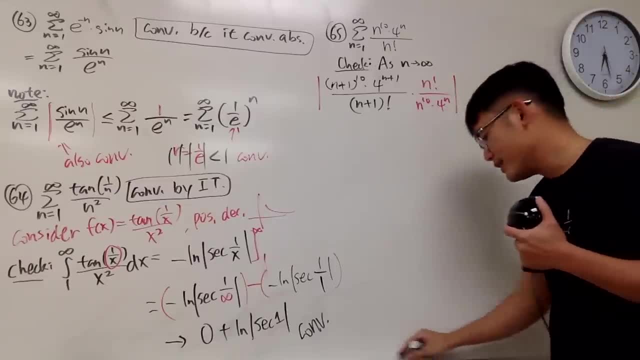 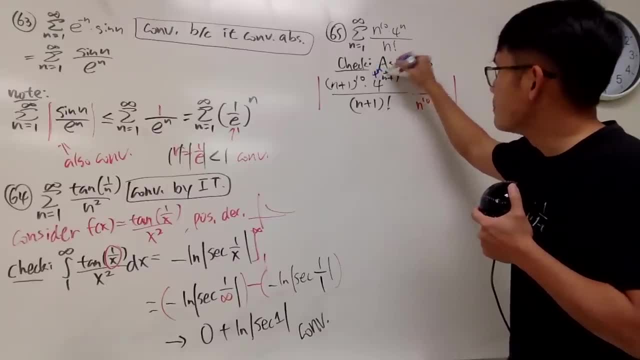 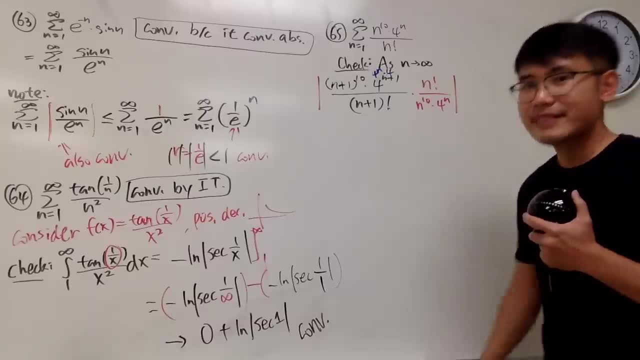 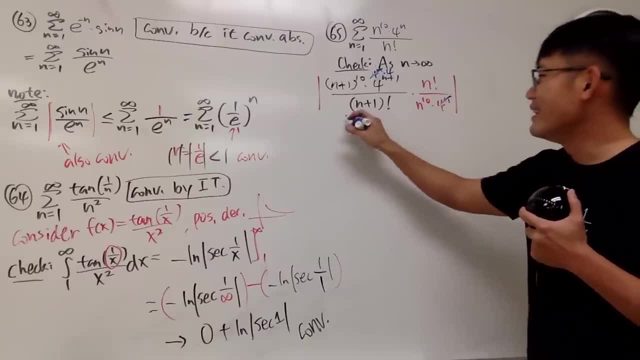 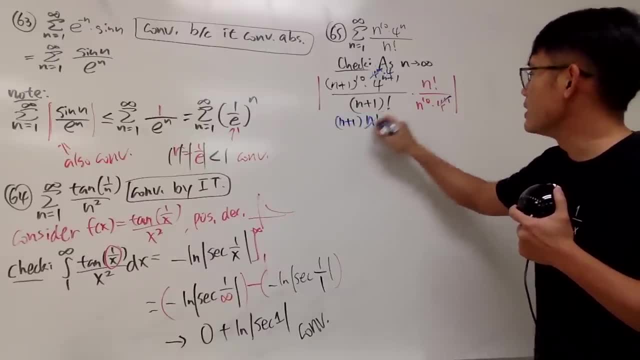 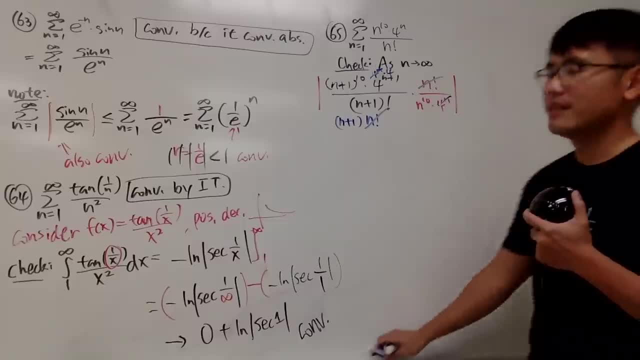 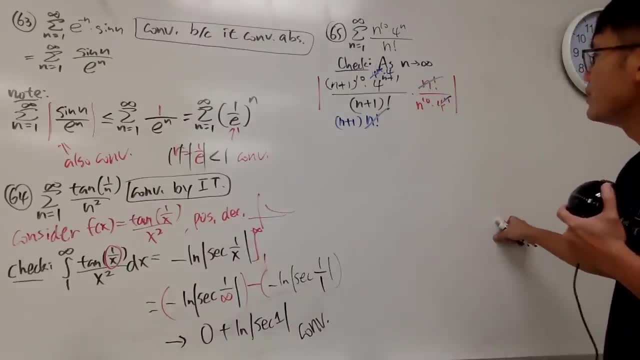 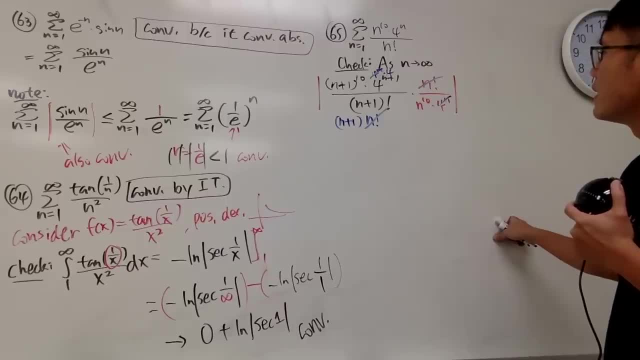 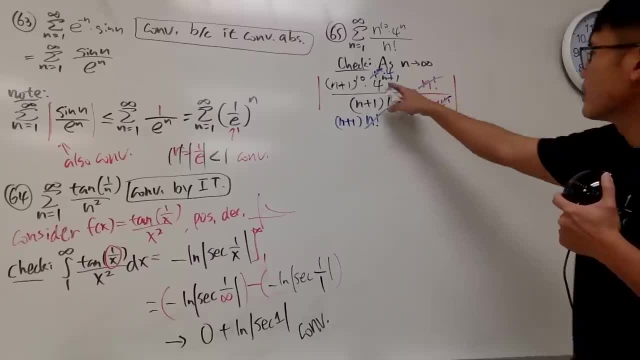 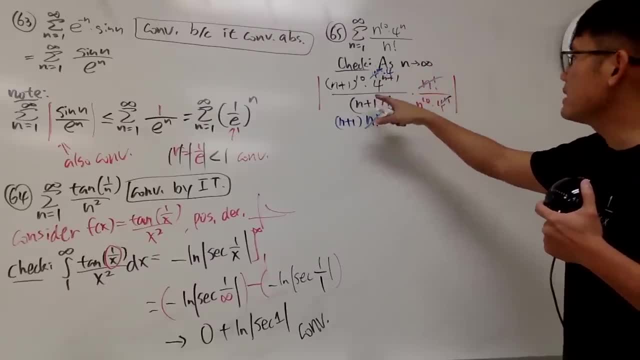 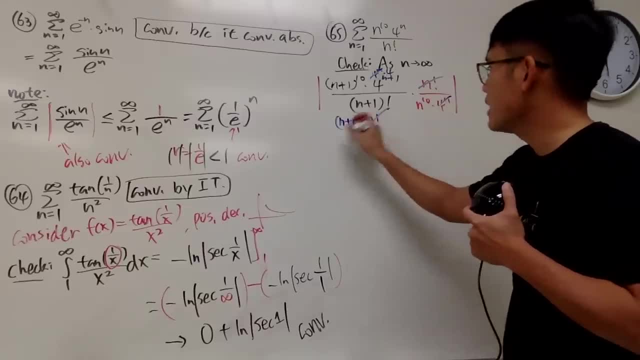 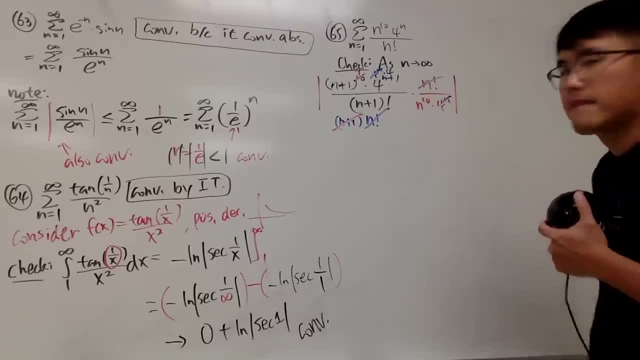 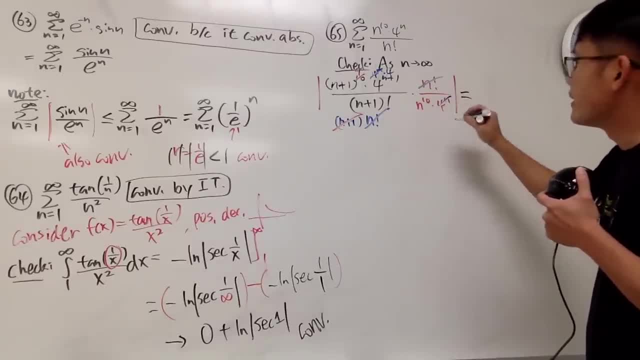 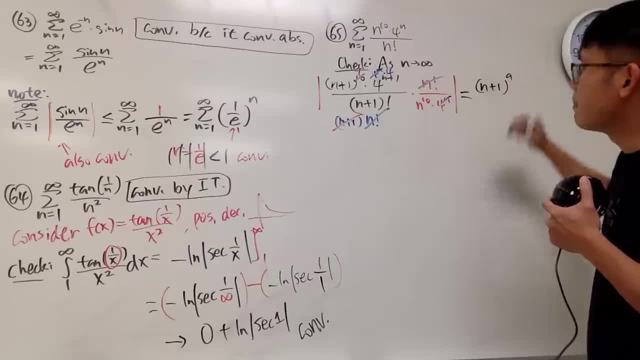 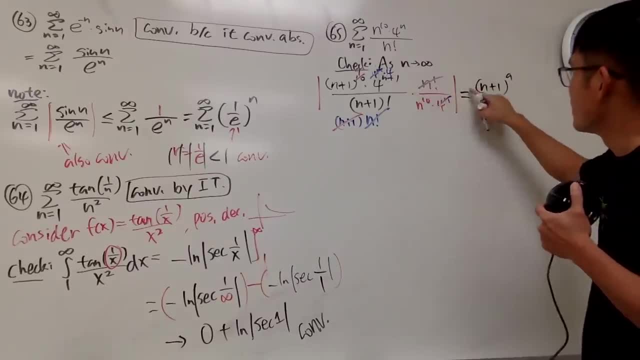 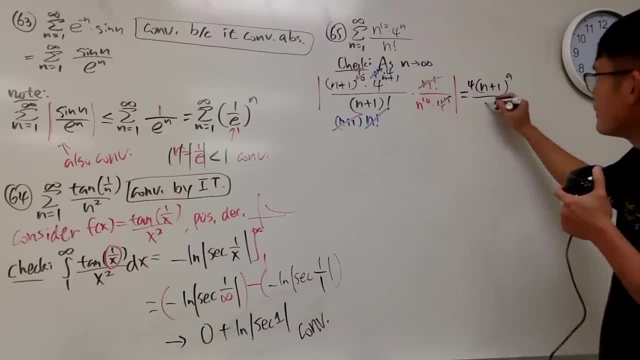 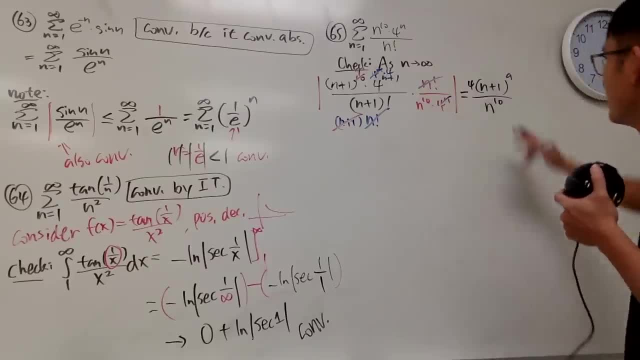 to the 10th power. this right here, power function over power sequence of all the power sequence for n to the, whatever it's power, this is finite, this is finite. but on the whole, this right here will give you zero, because the top is just going to be n to the ninth power times four. on the bottom we 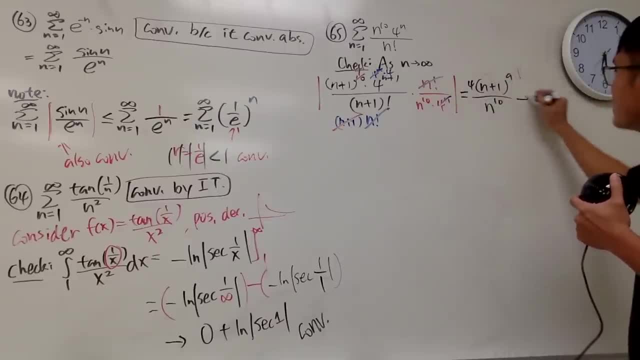 n to the- whatever It's power. This is finite, This is finite. But on the whole, this right here will give you 0.. Because the top is just going to be n to the 9th power times 4.. On the bottom we have n to the 10th. 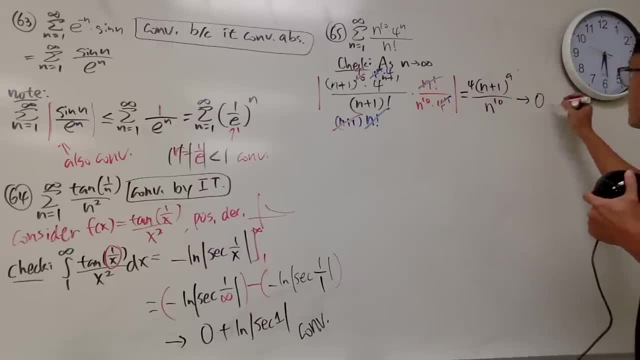 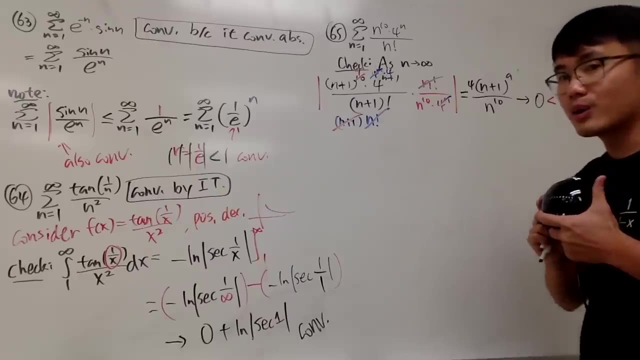 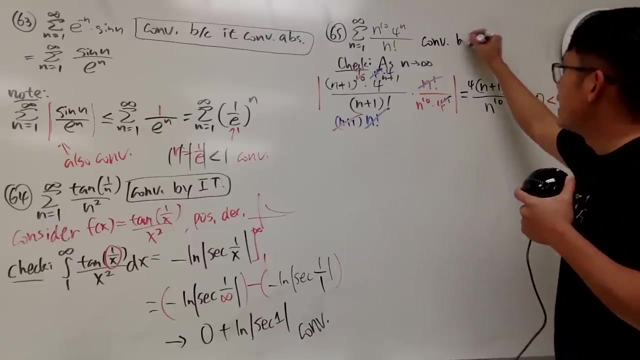 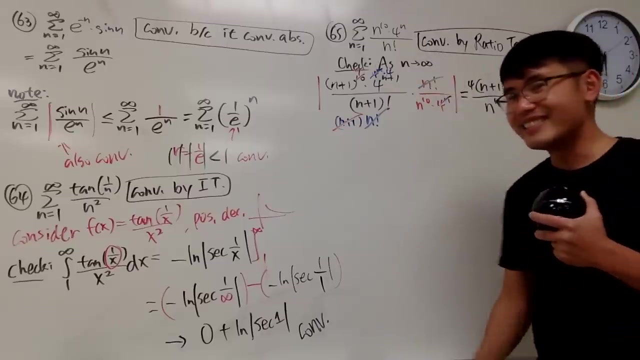 have n to the tenth, so this right here will be zero. it depends how you want to do. of course, this right here is less than one, so we can draw our conclusion and i will come back here and i will just tell you: this right here converges by the ratio test, by the ratio test, like that. 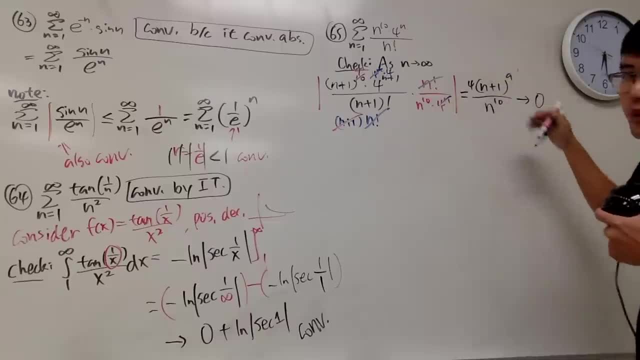 So this right here will be 0.. It depends how you want to do it, of course. This right here is less than 1.. So we can draw our conclusion And I will come back here and I will just tell you this right here: converges by the: 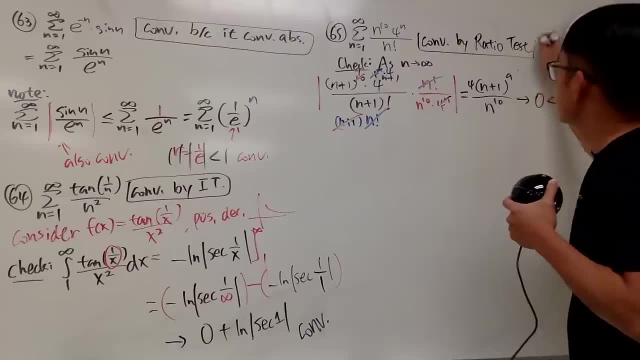 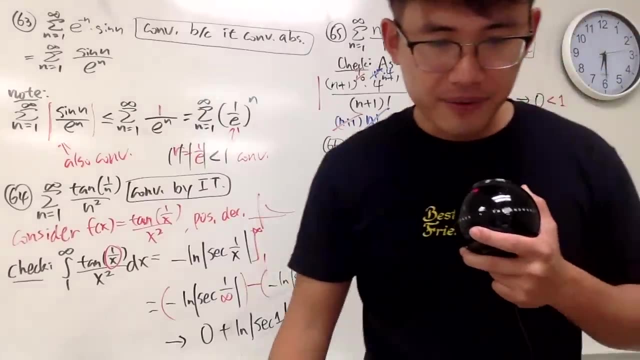 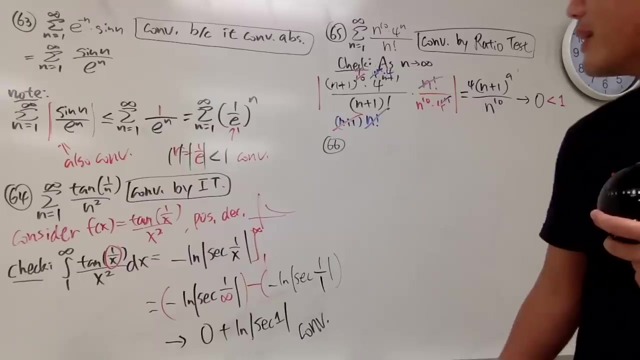 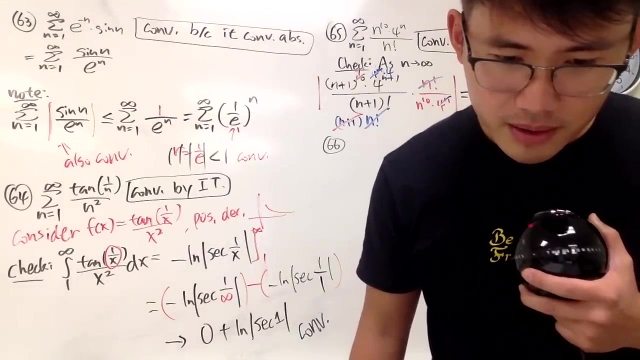 by the, by the ratio test, By the ratio test, Like that. Okay, now 65.. I mean 66.. Hmm, Wait, Wait, wait, wait, wait, wait. Oh, yeah, yeah, yeah. 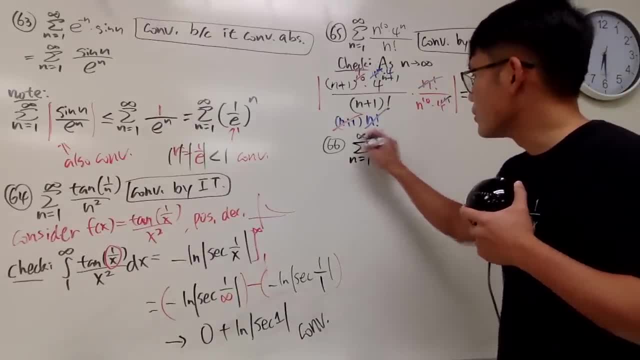 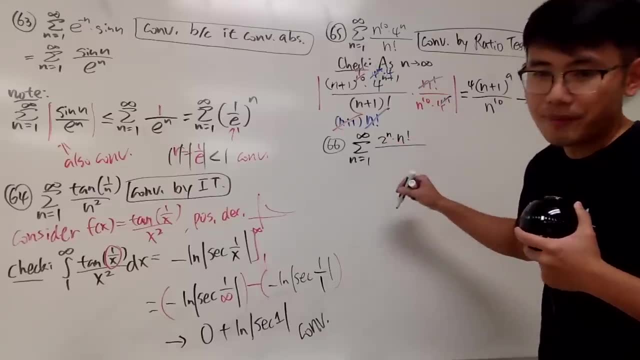 I'm not like missing any questions, or so. The sum as n goes from 1 to infinity, 2 to the- Now- this time we're fighting another one- 2 to the n times, n factorial over n plus 2 factorial. 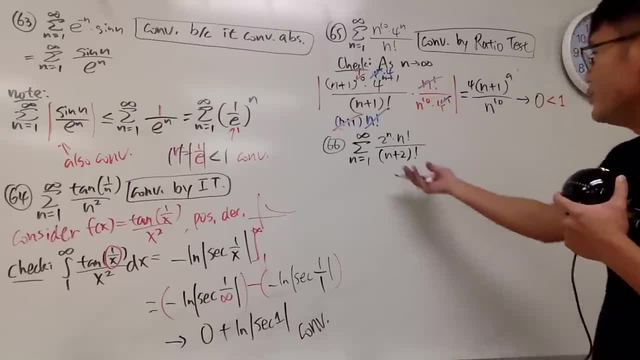 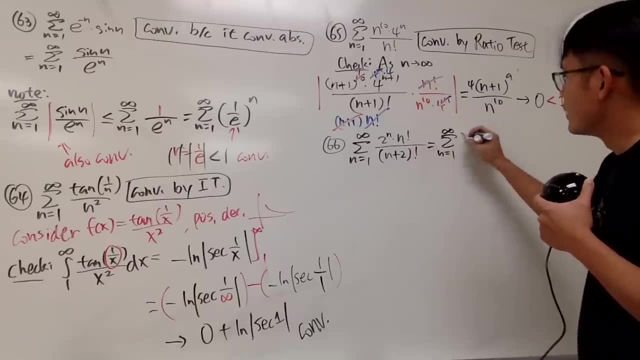 Hmm, Factorial fight, huh. And the truth is, you can actually simplify this before you go, So let me just show you This right. here is actually the sum as n goes from 1 to infinity, 2 to the n times n factorial. 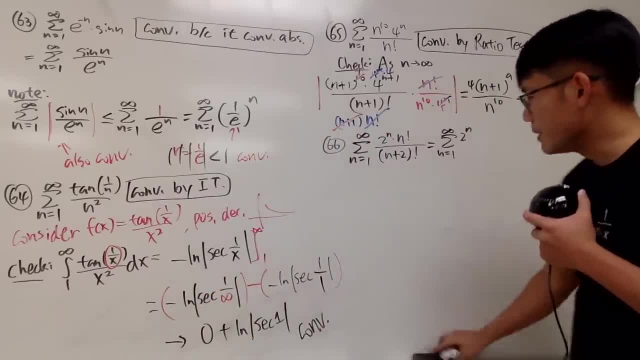 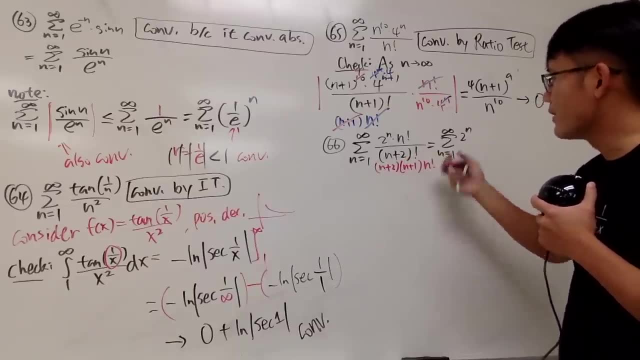 And actually let me just simplify it right here for you guys, Because right here we can write it as n plus 2, n plus 1.. And this is just n factorial. after that, This and that cancel out. So we actually have 2 to the n over, n plus 2, n plus 1.. 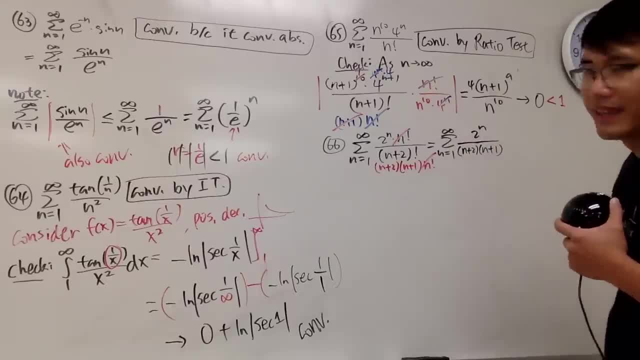 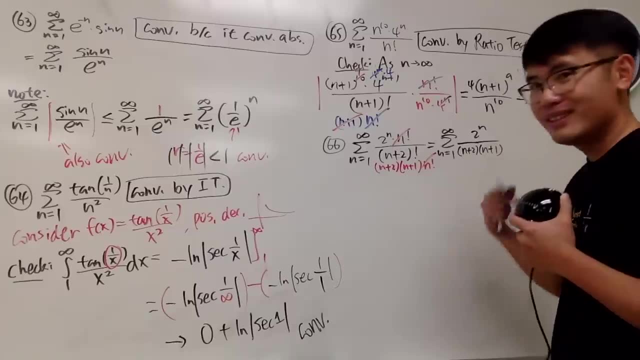 Like this, And of course, let's put a 2 to the n in the middle. Now, this right here actually has no competition with the denominator, Because the top is 2 to the n and the bottom is n squared, And of course you still have to just make this legitimate. 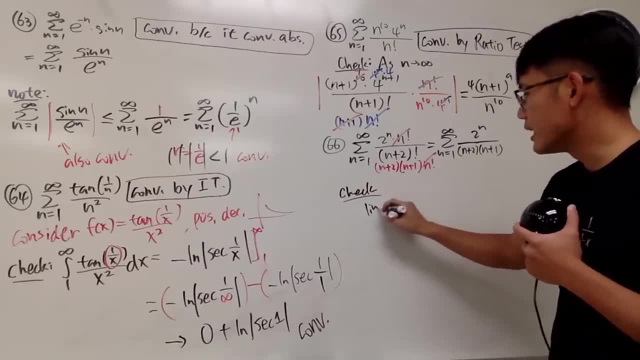 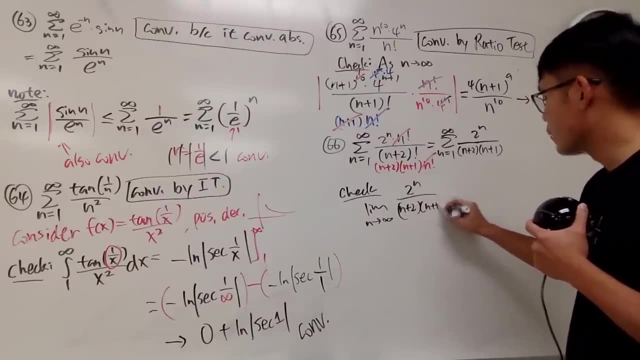 I will just tell you: Let's go ahead and show that. Just put this down The limit as n goes to infinity, 2 to the n over, n plus 2, n plus 1. That's at most like n squared on the bottom. 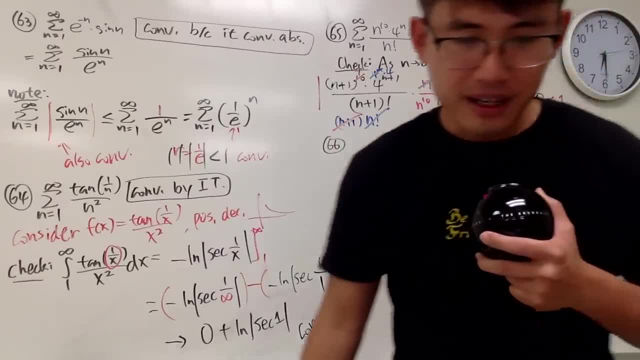 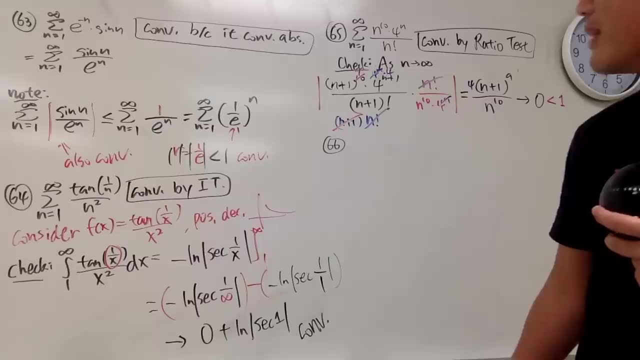 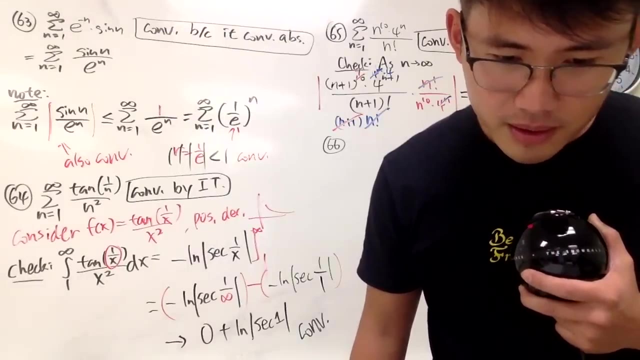 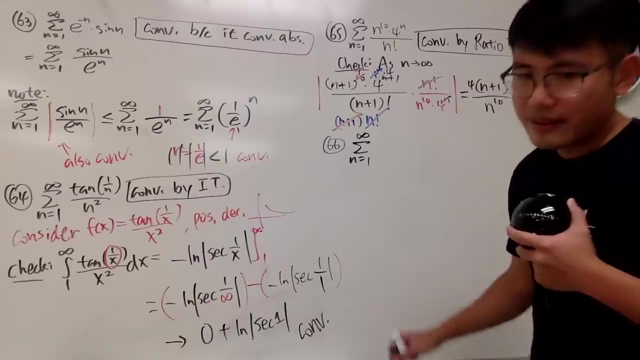 okay, now 65, i mean 66, wait, wait, wait, wait, wait. oh yeah, i'm not like missing any equations. also, the sum as n goes from one to infinity. two to the n. now, this time we're fighting another one. two to the n times n factorial over. 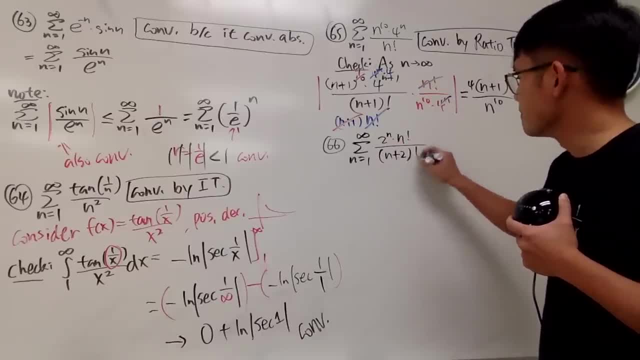 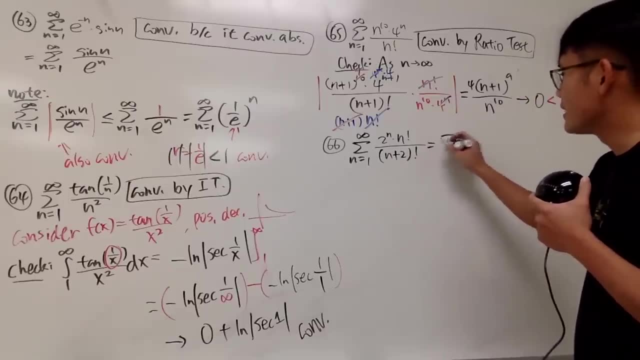 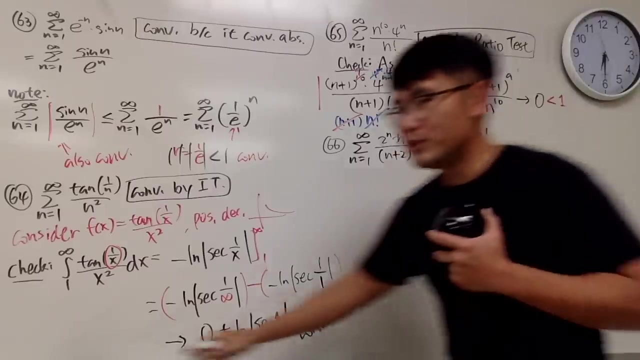 n plus two factorial factorial fight. huh, and the truth is, you can actually simplify this before you go, so let me just show you this right. here is actually the sum as n goes from one to infinity, two to the n times n factorial. and actually let me just simplify the. 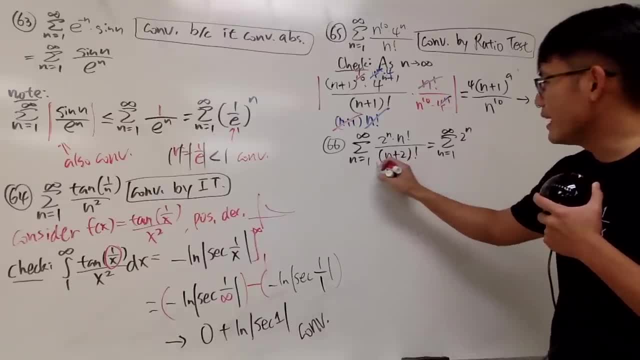 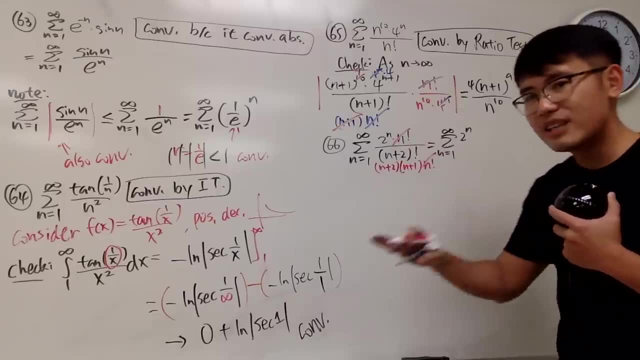 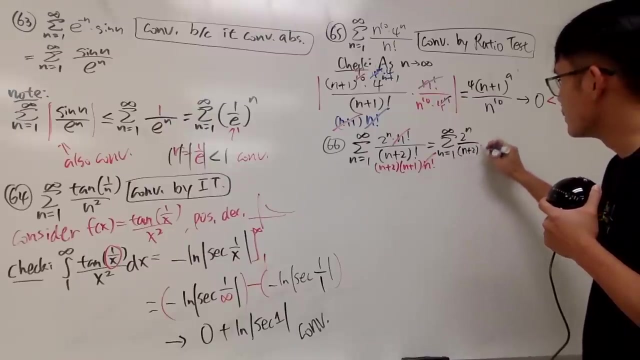 right here for you guys, because right here we can write it as n plus two, n plus one, and this is just n factorial. after that, this and that cancel out. so we actually have two to the n over, n plus two, n plus one, like this, and of course let's put a two to the n in the middle. now this: 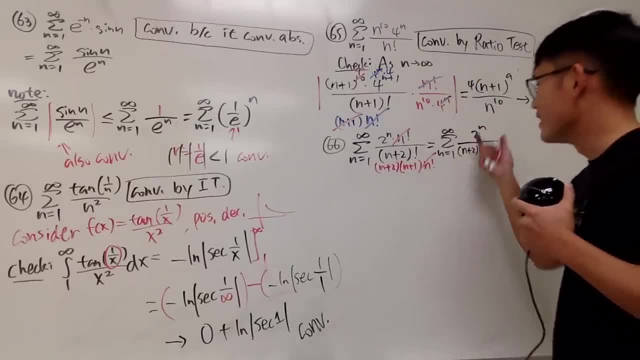 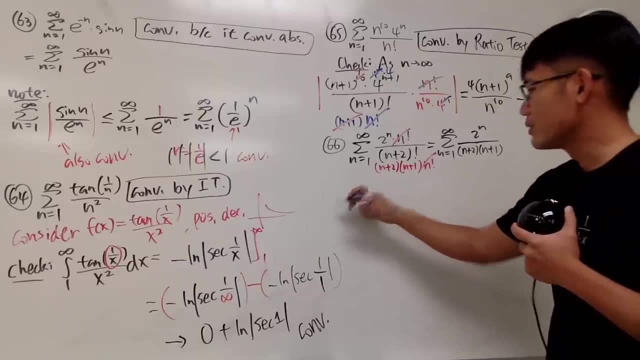 right here actually has no competition with the denominator, because the top of the top, the top is two to the n and the bottom is like n square. and of course you still have to just make this legitimate. i will just tell you: let's go ahead and show that. just put this down the limit as 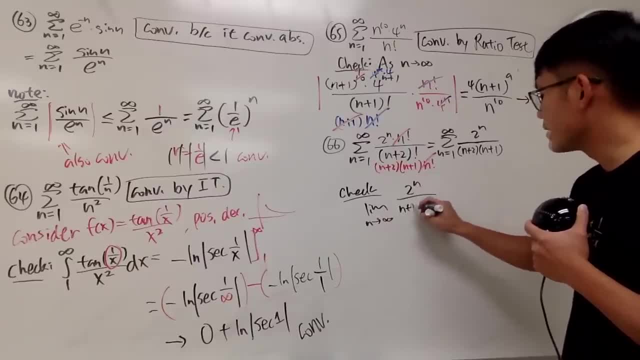 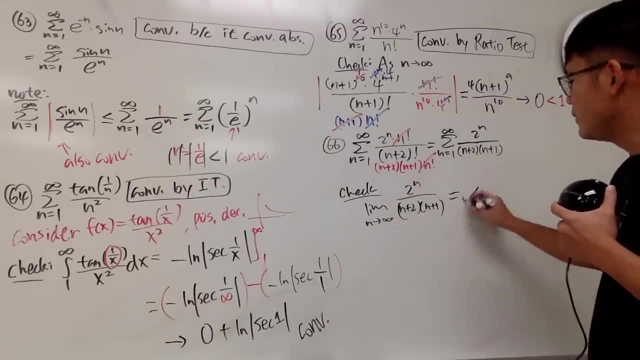 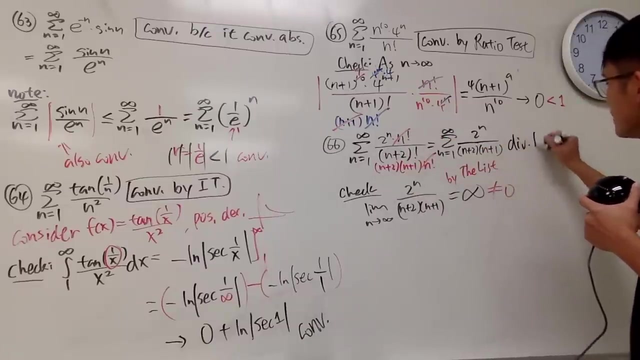 n goes to infinity, two to the n over, n plus two, n plus one, that's at most like n square on the bottom. but this, right here, it will actually give you infinity. why, by the list? and this is so good? because infinity is of course zero. so we can come back here and say: this guy diverges by tfd, right, tfd, and we are done very. 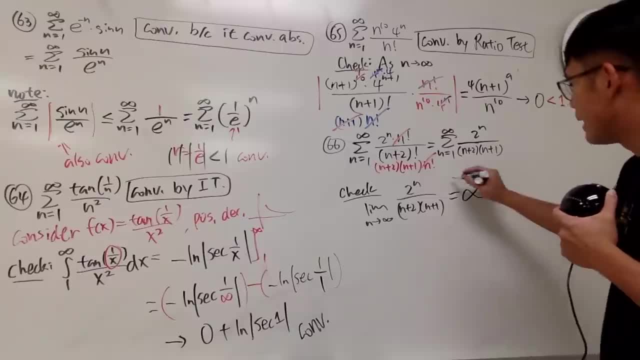 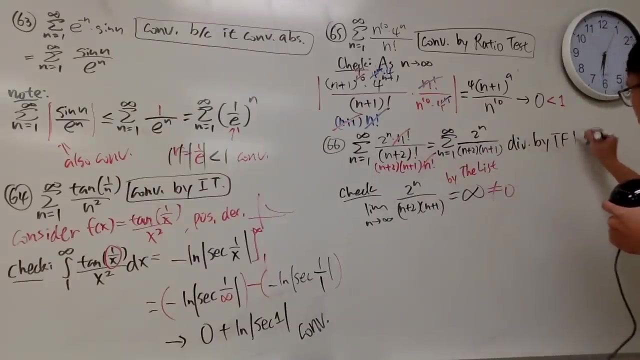 But this right here, it will actually give you infinity. Why By the list? And this is so good? because infinity is, of course, not 0.. So we can come back here and say: this guy diverges by tfd, Tfd, right. 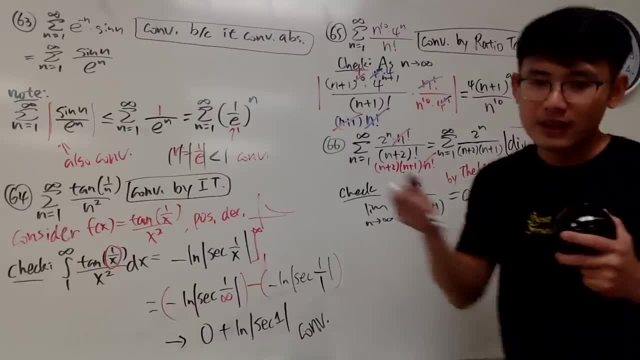 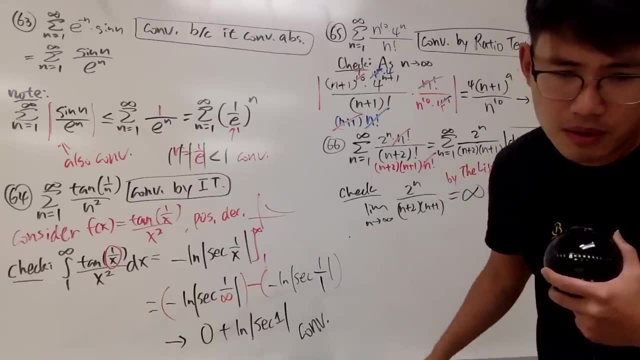 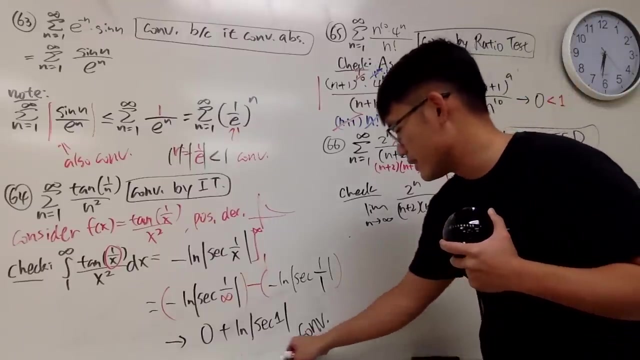 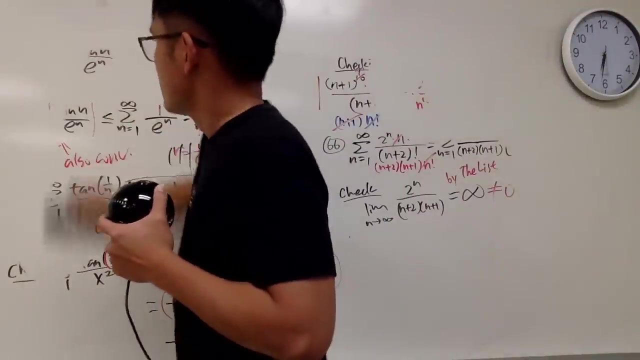 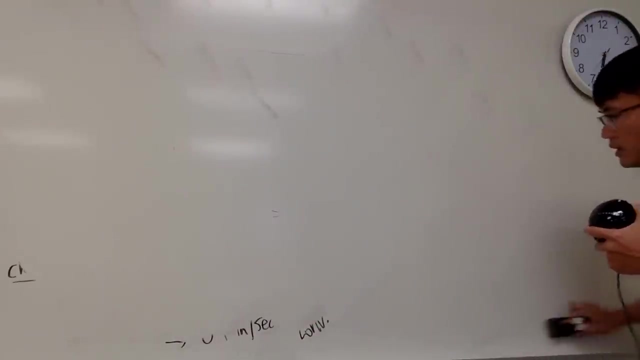 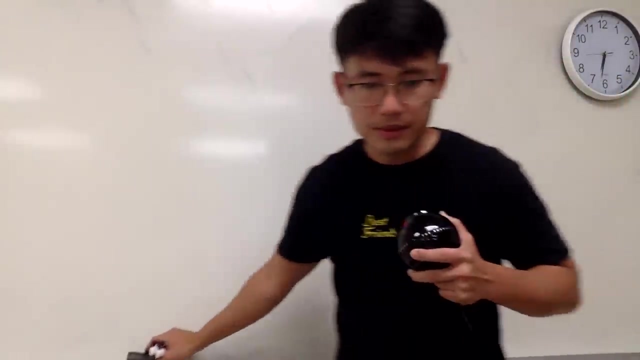 Tfd And we are done. Very, very cool. Now I will fit in another one. Remember, actually, let's see, Actually I will just erase this right here. Actually, I need to use my phone a little bit. 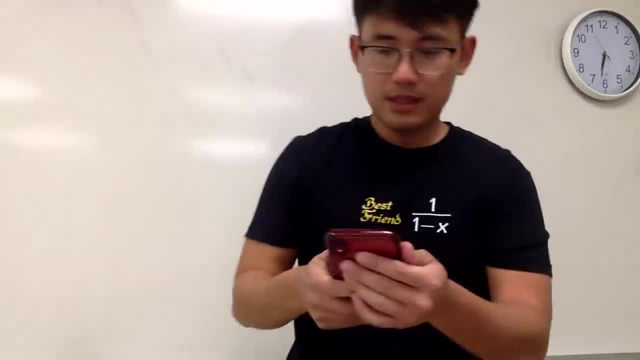 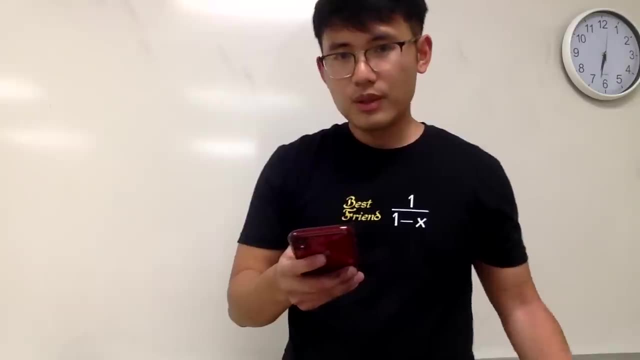 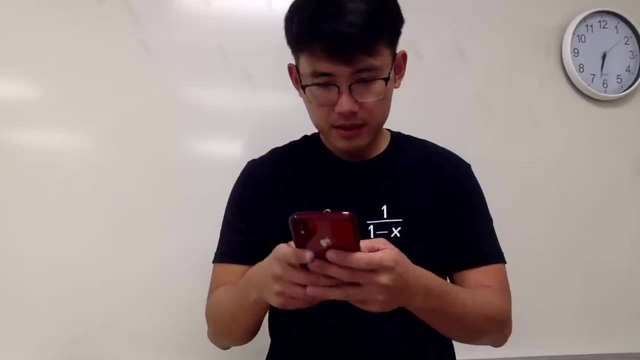 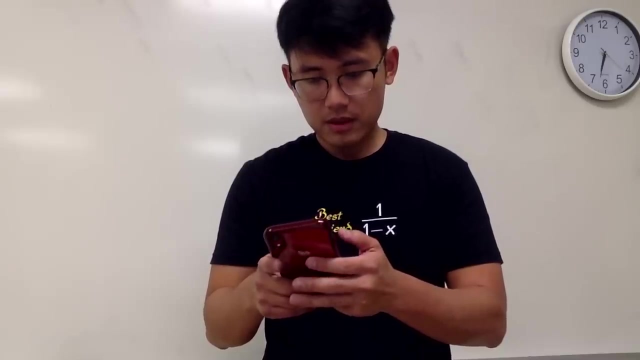 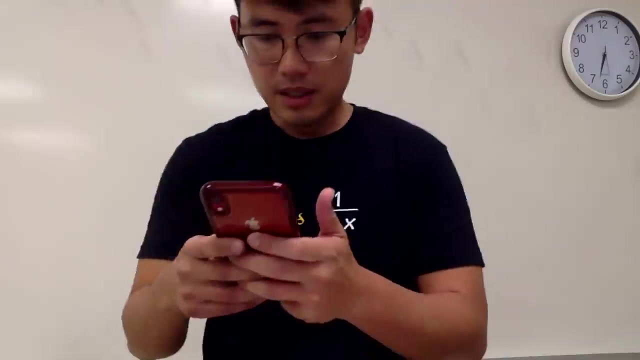 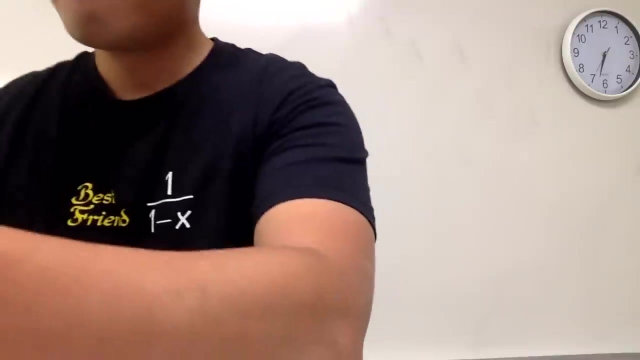 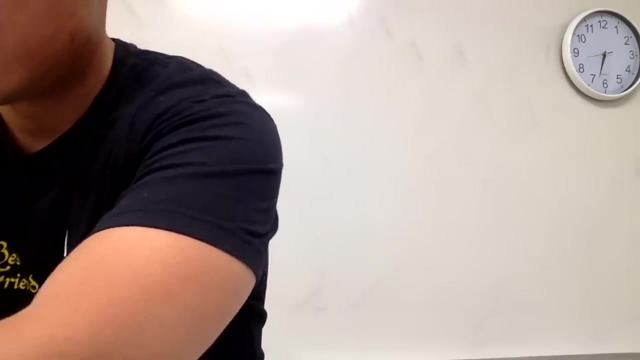 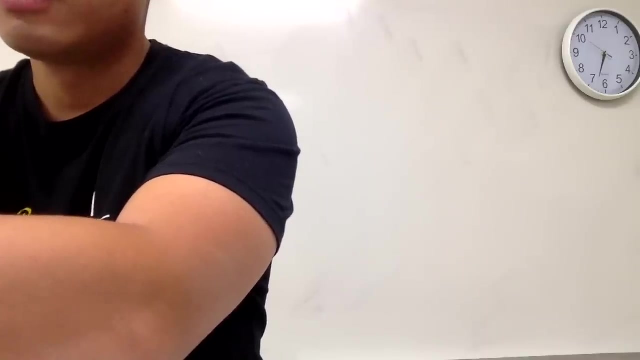 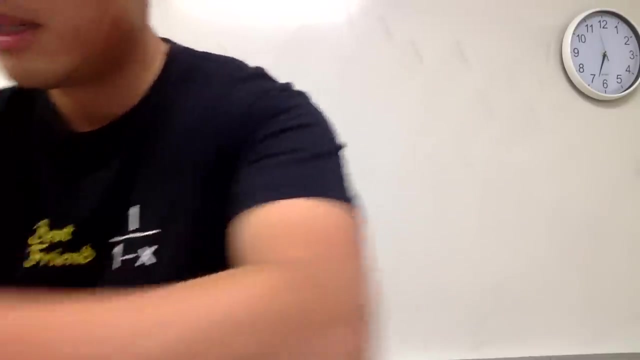 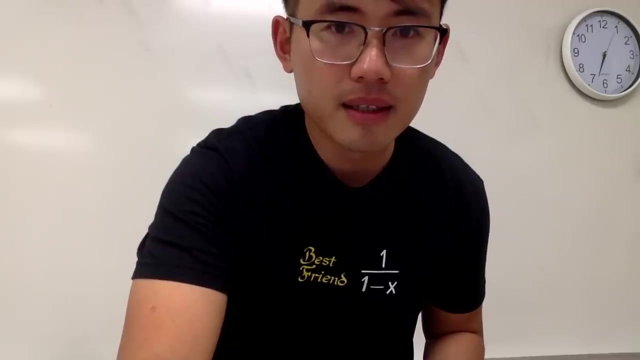 Okay, Oh, Workout man, different kind of workout. And then I'm going to make sure I can also still record this right here. And then I'm going to make sure I can also still record this right here. And then I'm going to make sure I can also still record this right here. 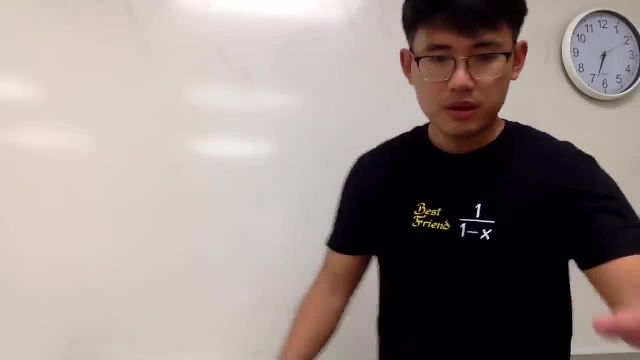 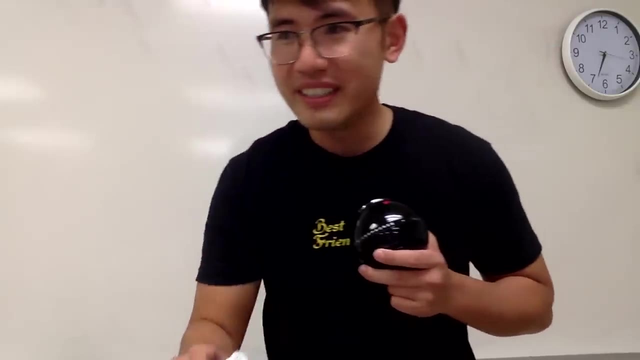 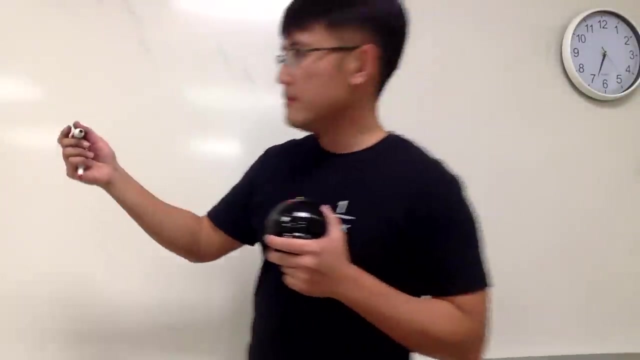 Alright, Alright, So that was number 66. So that was number 66. Now number 67. Now number 67. Let's just double check if the board is clean enough. Let's just double check if the board is clean enough. Okay, Number 67, right here. 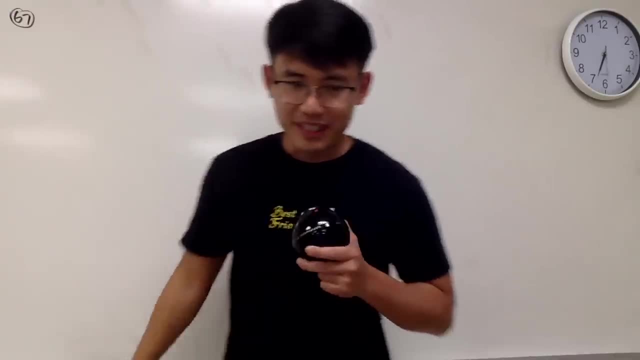 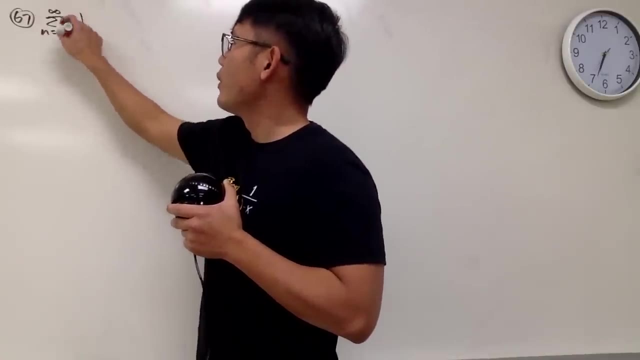 Okay, number 67. It's a fun one again. Oh man, not really Okay. the sum As n goes from 1 to infinity. 1 over square root of n factorial. 1 over square root of n? factorial. Wow, we put the n? factorial inside of the square root. 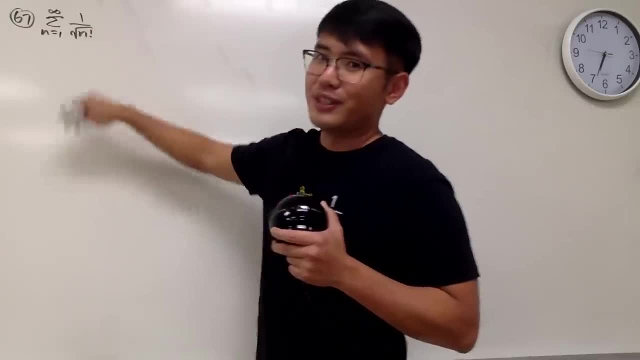 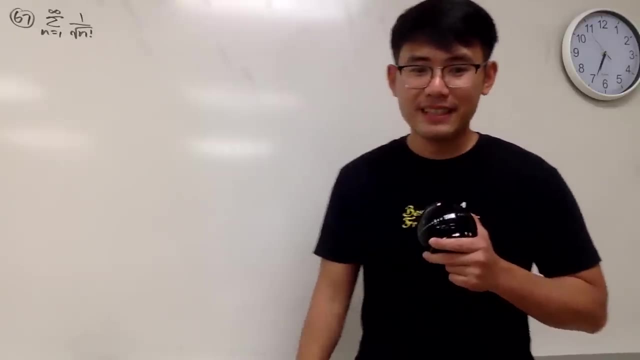 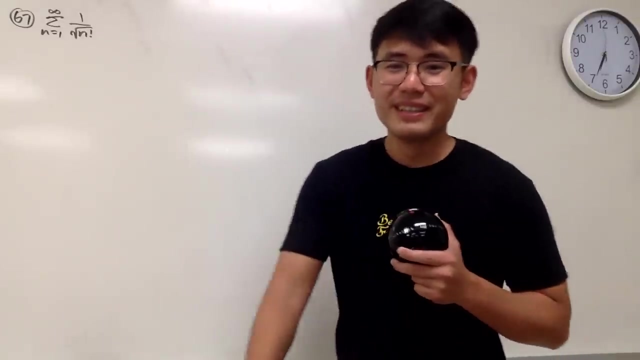 As you all know, 1 over square root of n diverges, But 1 over n factorial converges. So we put it together inside. Let's see what will happen. Alright, Let's see, maybe we can. I'm not looking at any notes, I'm just looking at the question. 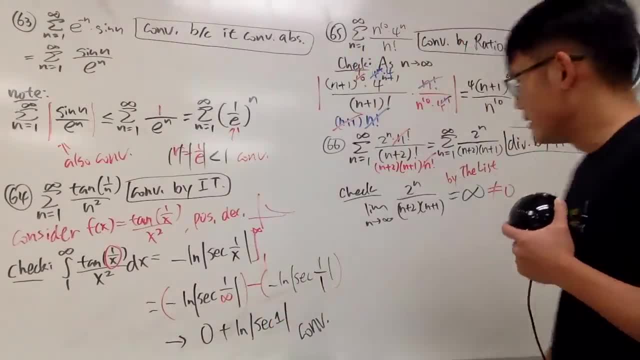 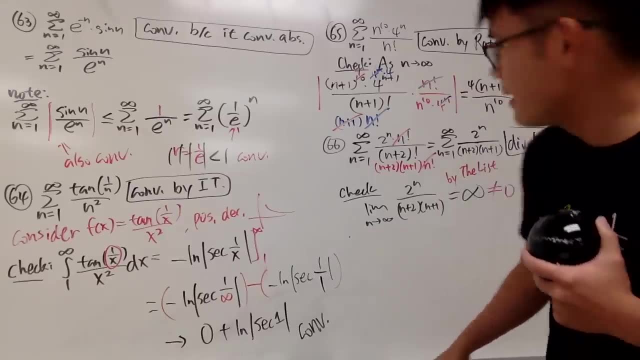 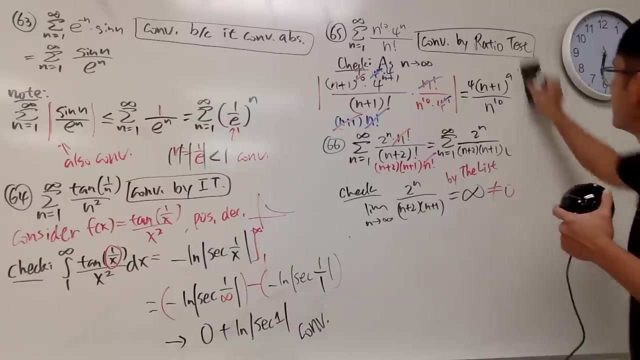 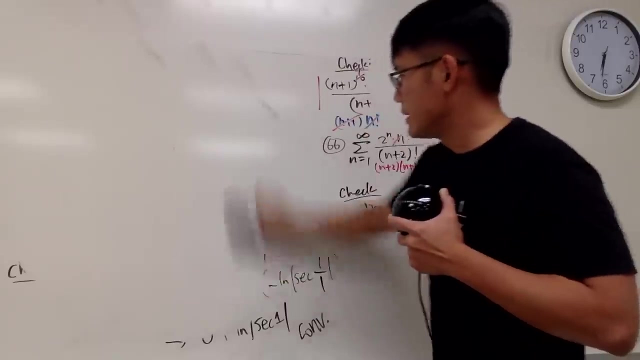 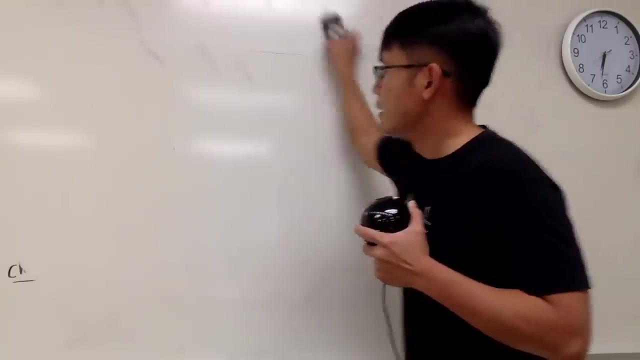 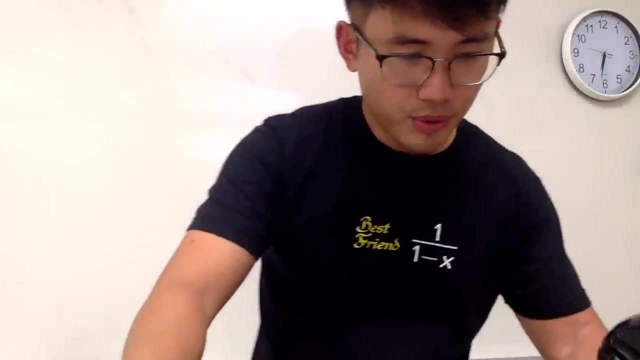 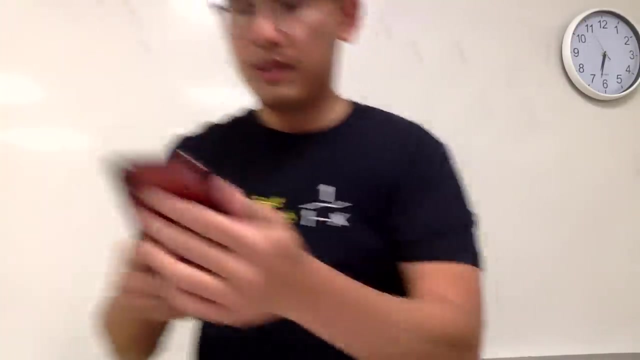 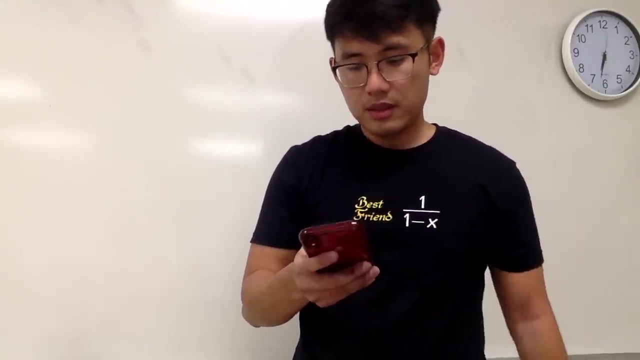 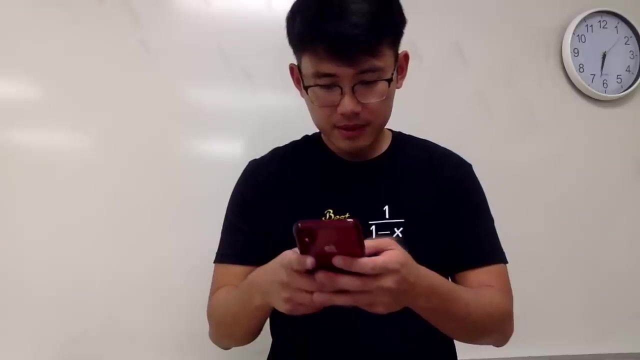 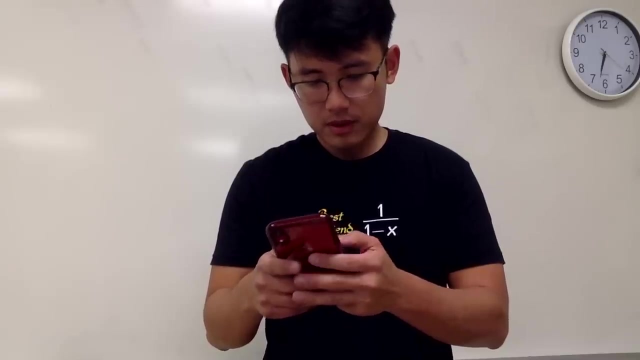 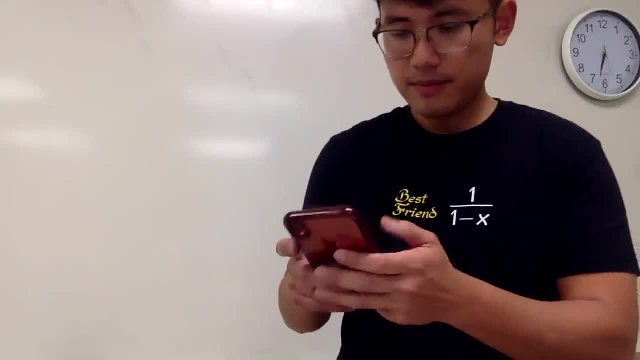 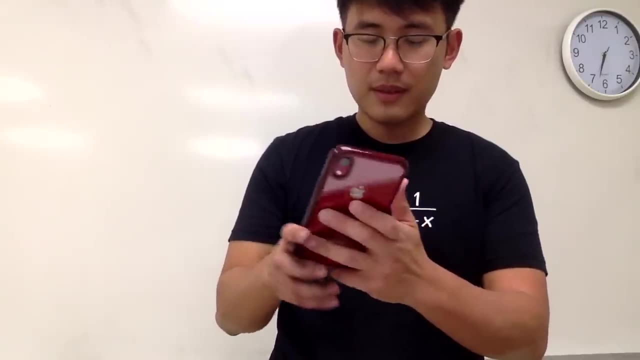 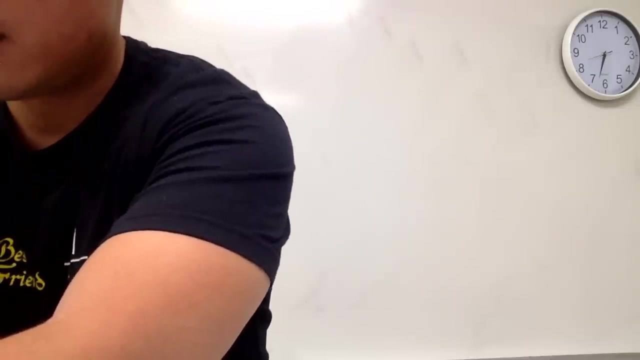 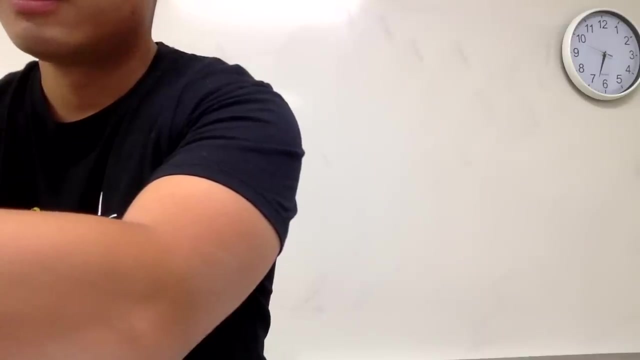 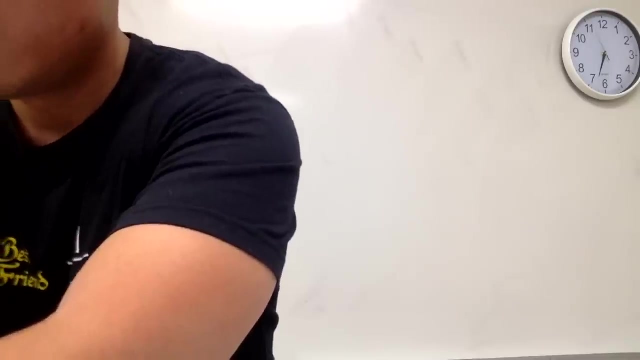 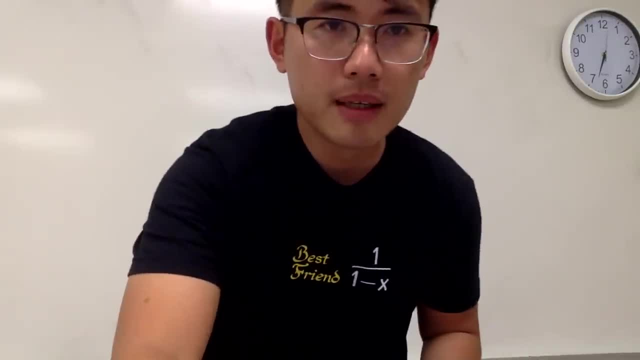 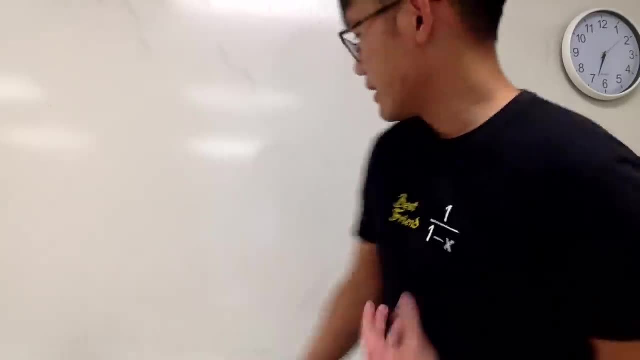 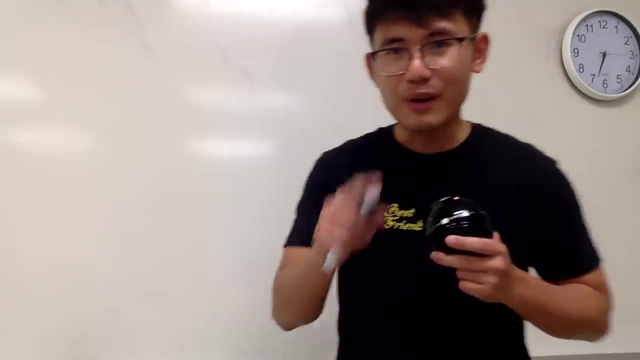 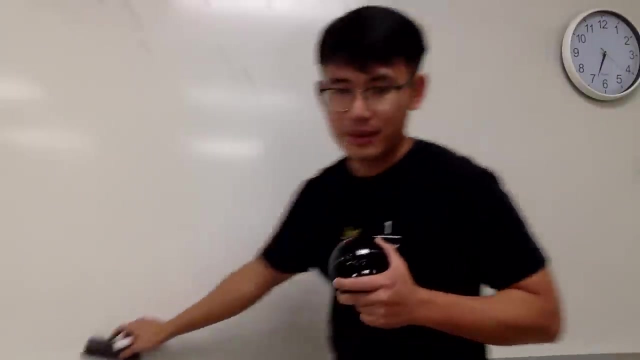 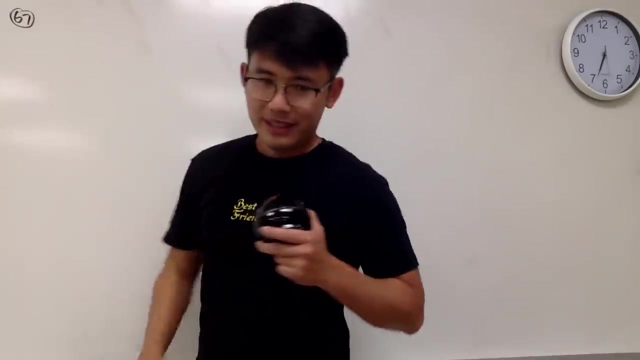 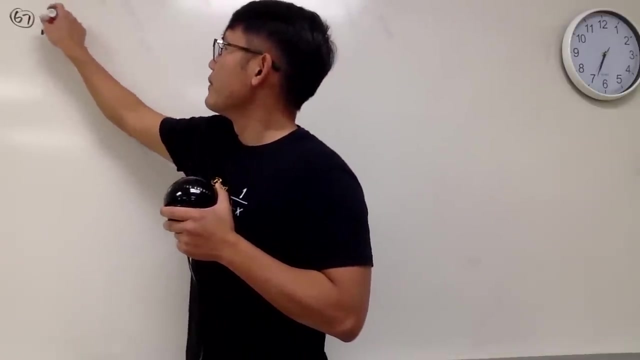 All right, so that was number 66, now number 67, let's just double check if the board is clean enough or not. okay, number 67, right here. okay, number 67, it's the fun one again. oh man, not really okay. the sum as n goes from 1 to infinity: 1 over square root of n, factorial. 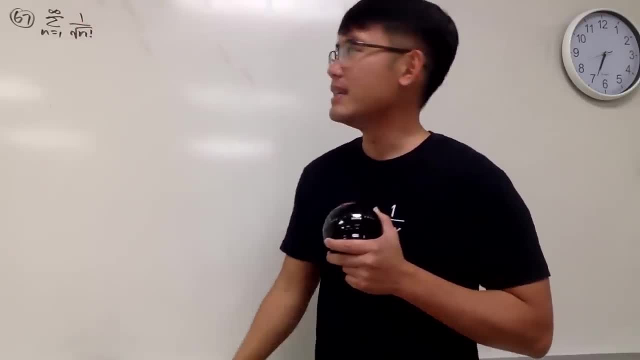 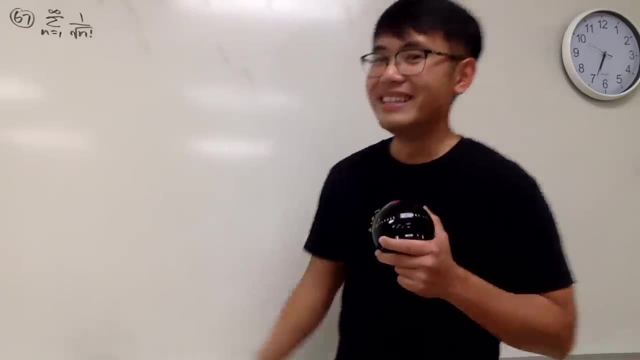 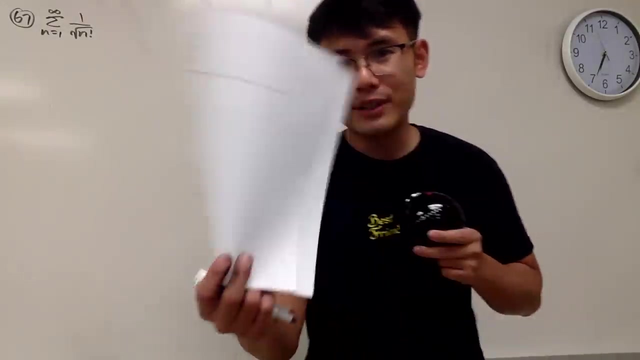 wow, we put the n factorial inside of the square root. as you all know, 1 over square root of n diverges, but 1 over n factorial converges, so we put it together inside. let's see what will happen. all right, let's see, maybe we can. well, I'm not looking at. 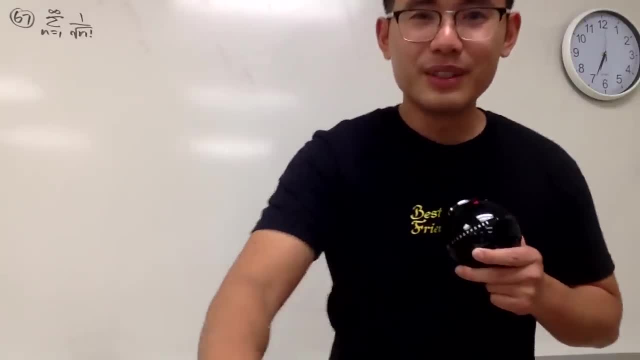 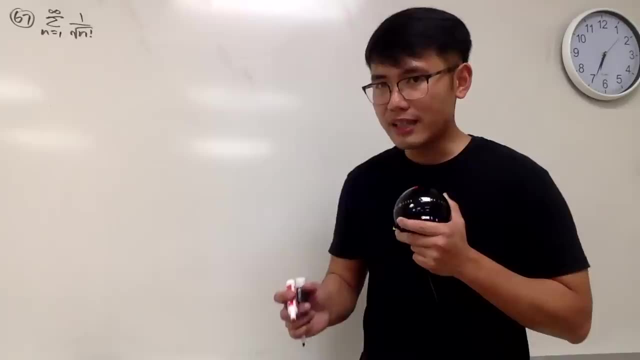 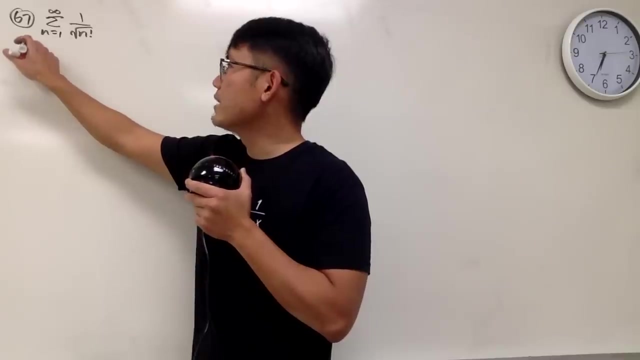 any notes? I'm just looking at the question to see what we can do with that right. all right, maybe we can try with the ratio test. why not? because when you have square root it's like power, so that's very nice. so I will just go ahead and use the ratio test. so here we go. check s. 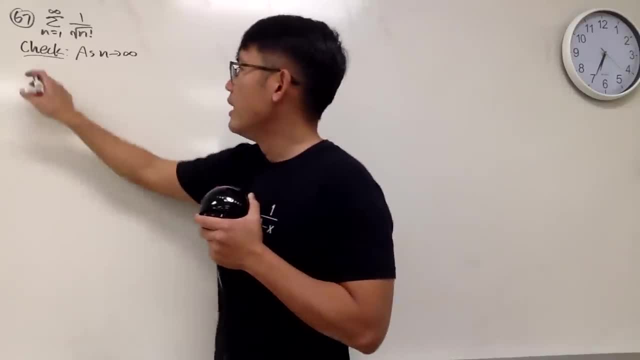 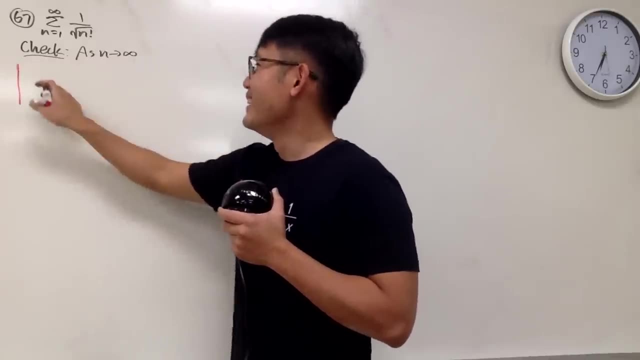 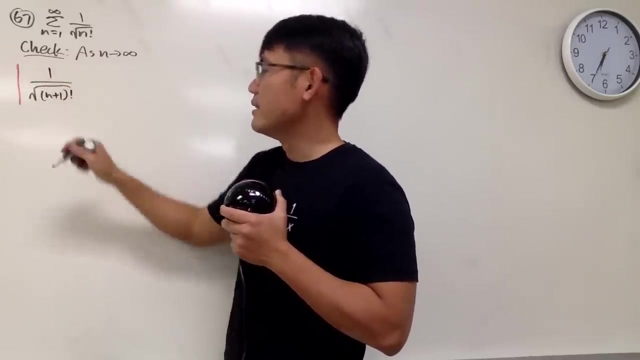 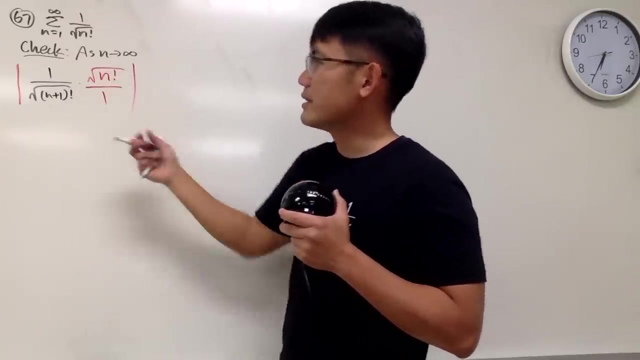 n goes to infinity, n? t. okay, take the absolute value, but you really don't need to anyway. the first one is 1 over square root of parentheses n plus 1 factorial, and you do the reciprocal of that which is square root of n factorial over 1, like this: 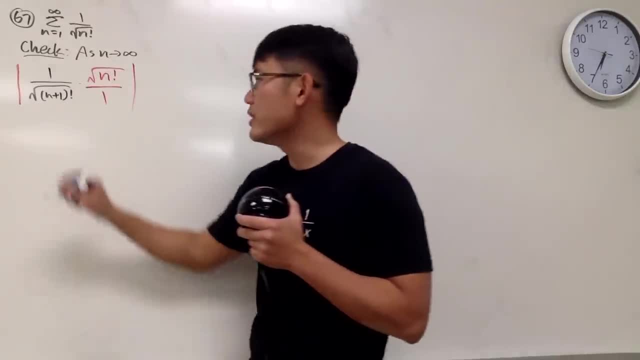 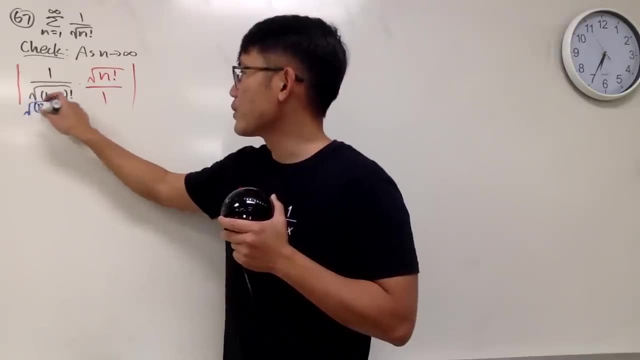 and now we are going to just have some fun with the cancellations. this, right here again, is n plus 1, times n factorial. and don't forget, this is the square root of this, square root of that, because they're all positive, that's nice, and of course we can cancel this and that. 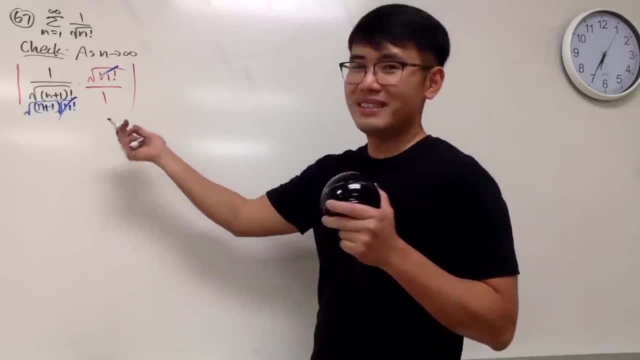 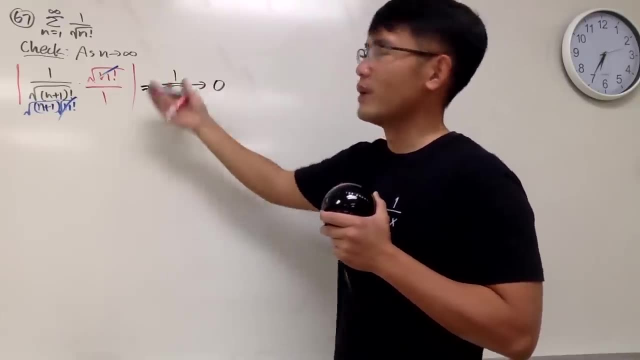 that's so wonderful. look at that. what's this now? it's just equal to 1 over square root of n plus 1, and of course this will go to 0 as n go to infinity. this is the ratio test, so 0 helps. 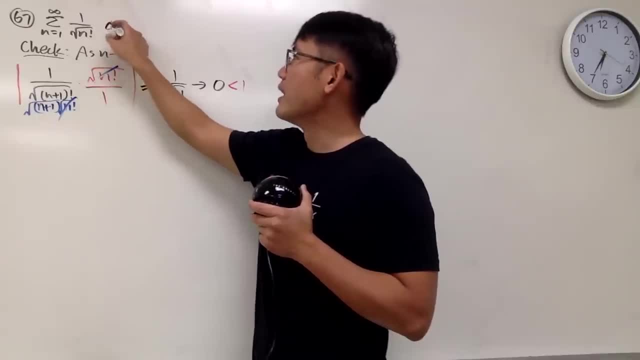 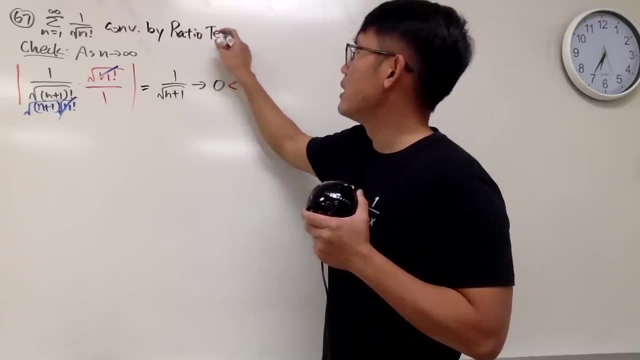 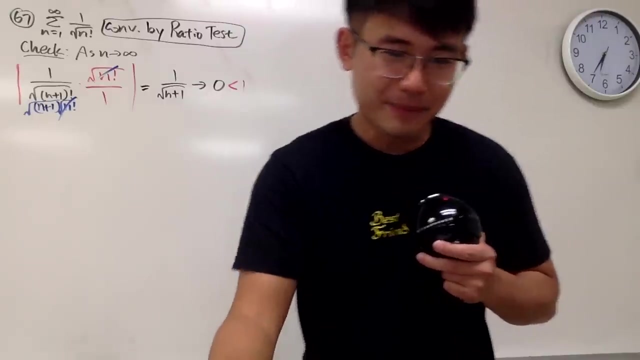 this is less than 1, so we can come back here and say this right here. third is by the ratio test. I won't. I almost wanted to say by ratio, but like, ratio is not a person. okay, now, that was number 67,, not 60,. 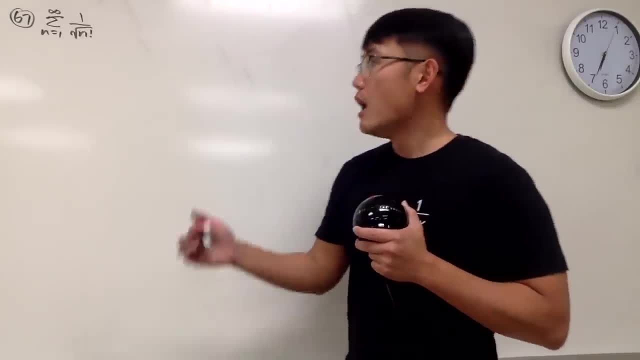 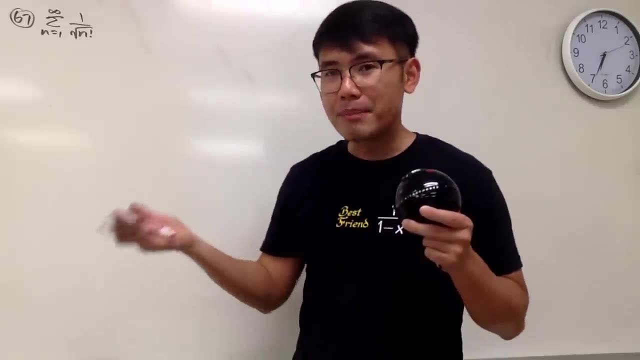 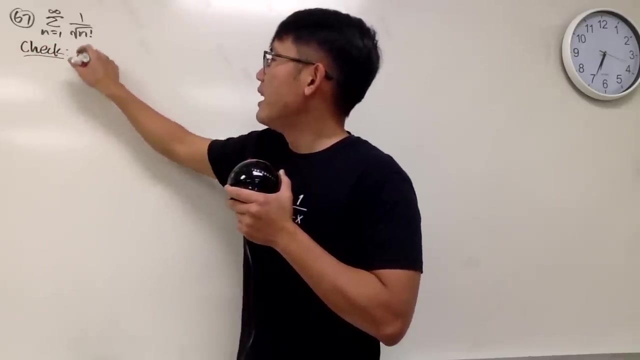 To see what we can do with that. Alright, Maybe we can try with the Ratio test. Why not? Because when you have square root, it's like power, So that's really nice. So I will just go ahead and use the ratio test. So here we go. 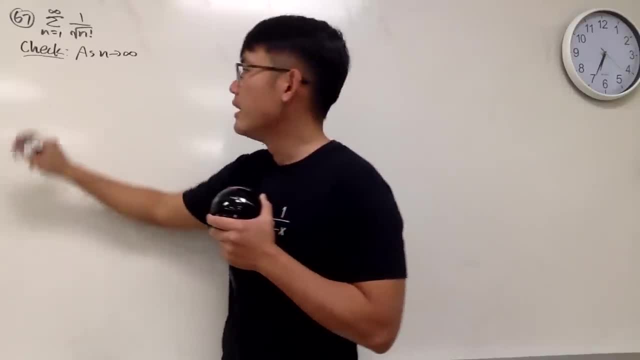 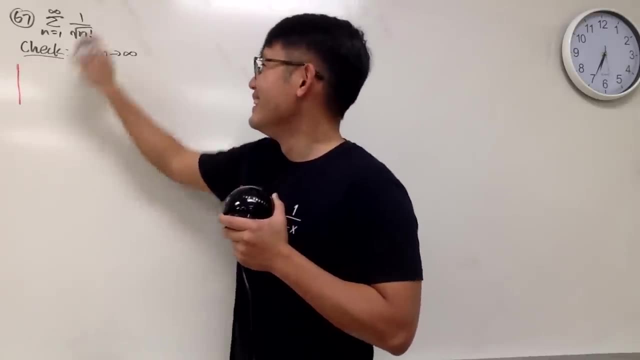 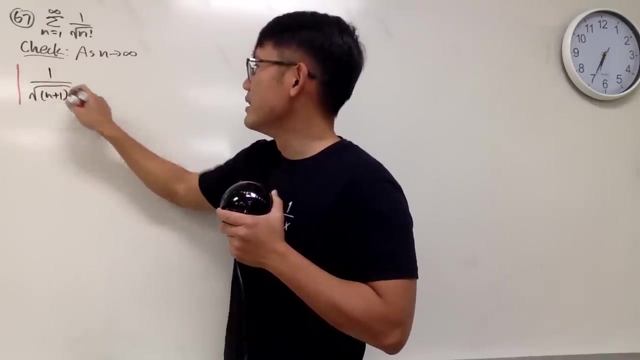 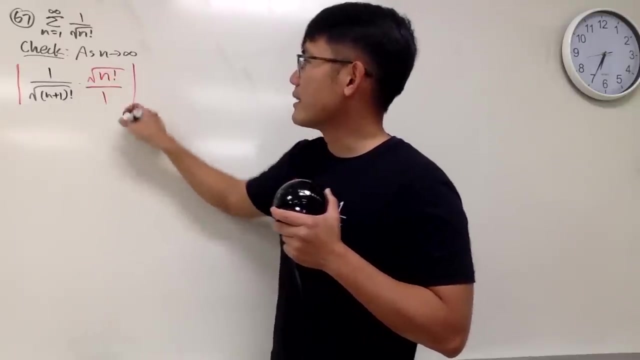 Check s And goes to infinity. Okay, Take the absolute value, But you really don't need to, Anyway, Anyway. So this is the square root of n factorial And you do the reciprocal of that, Which is square root of n factorial Over 1, Like this: And now we are going to. 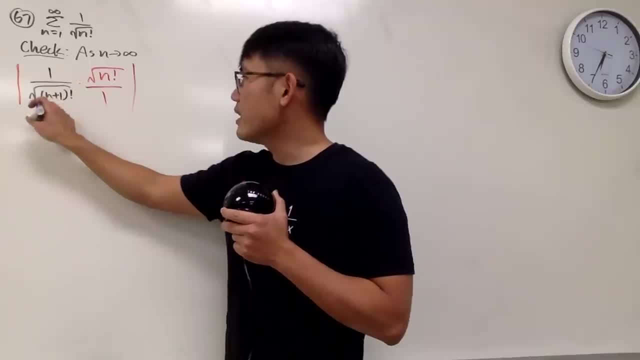 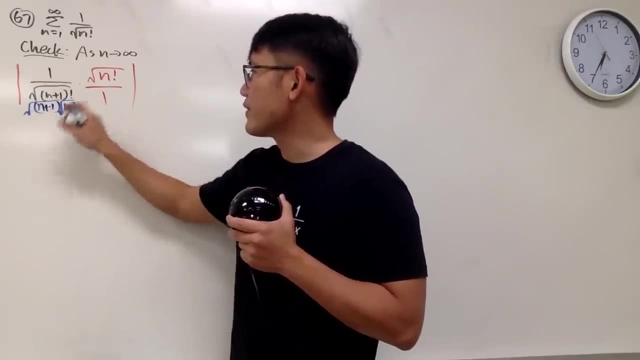 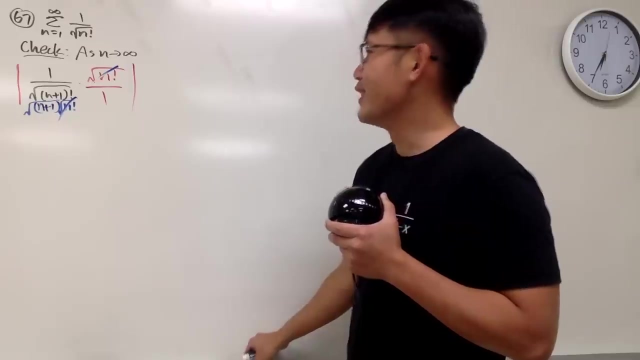 Just have some fun with the cancelation. This, right here again, is n plus 1 Times n factorial. And don't forget, this is the square root of this, Because they are all positive, That's nice, And of course we can cancel this and that That's so wonderful. 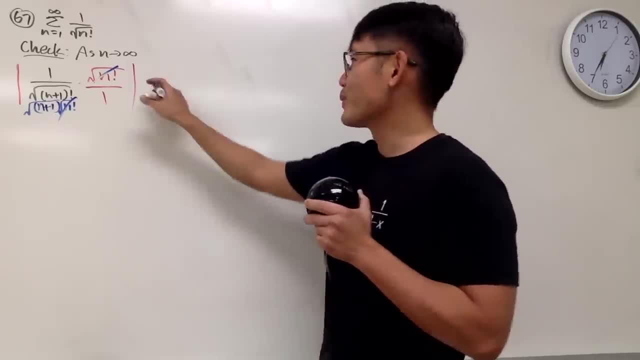 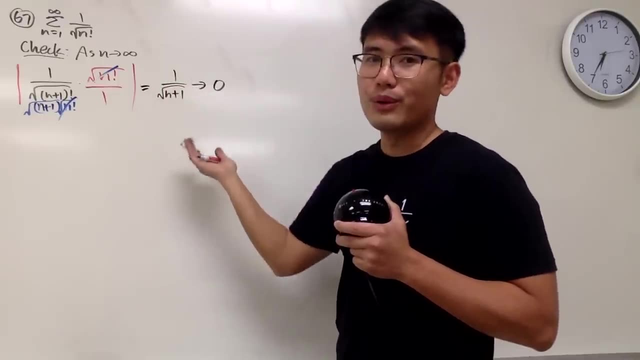 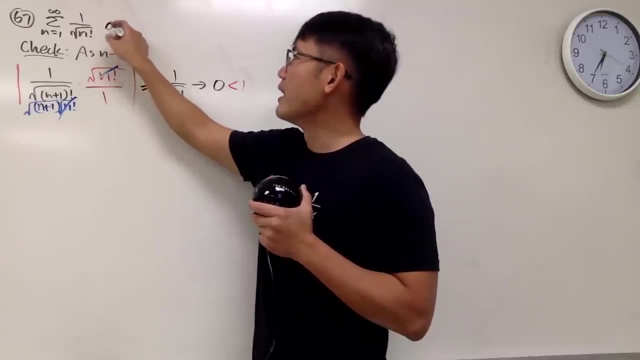 Look at that. What's this now? It's just equal to 1 over square root of n plus 1, And of course this will go to 0 And go to infinity. This is the ratio test. So 0 helps. This is less than 1. 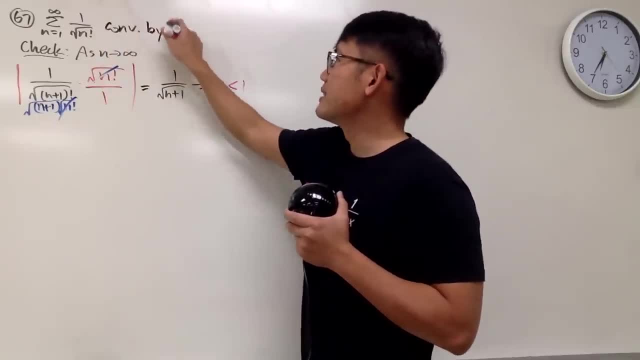 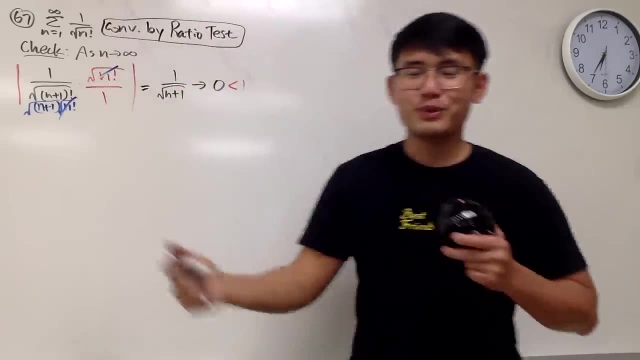 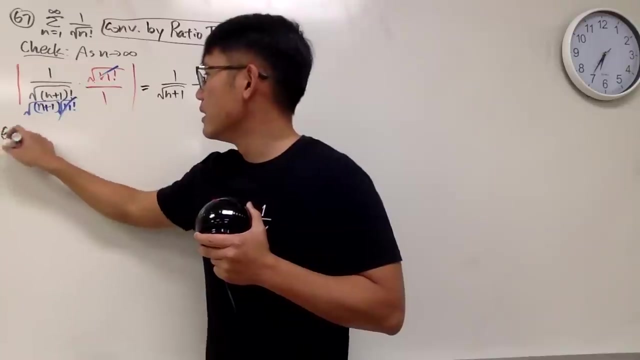 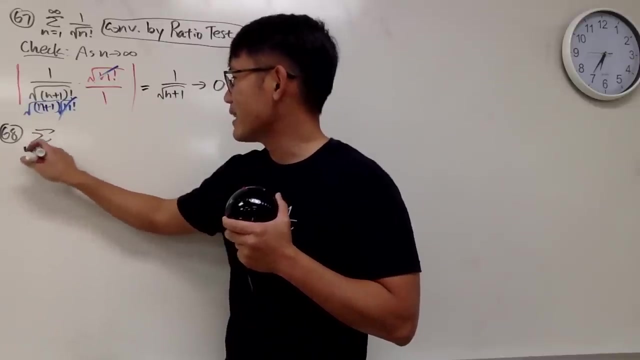 So we can come back here and say This right here: Converges by the ratio test. I want, I almost wanted to say by ratio. Okay, Now, that was number 67, Not 60. We are putting the Factorial into natural log. So sum as n goes from 1 to infinity. 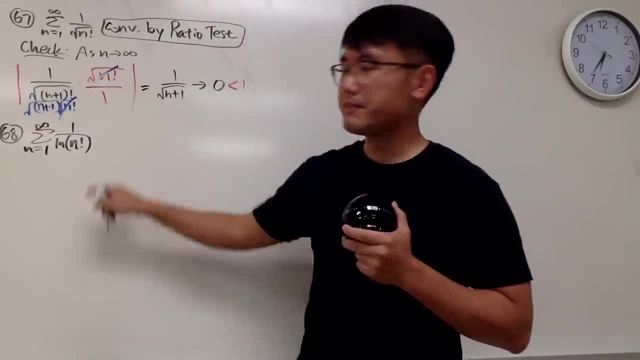 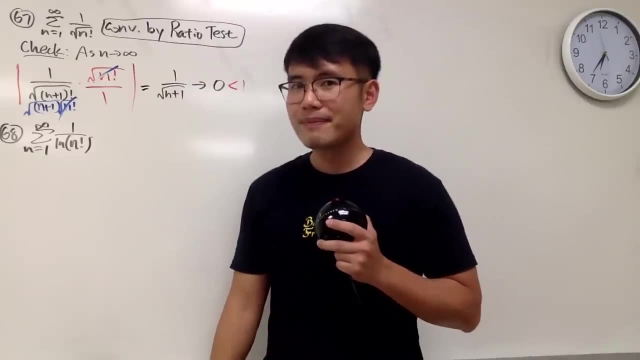 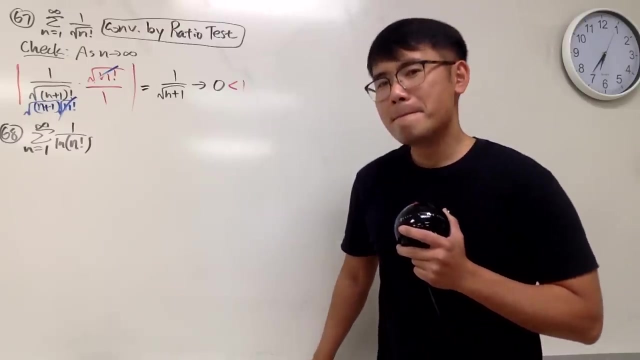 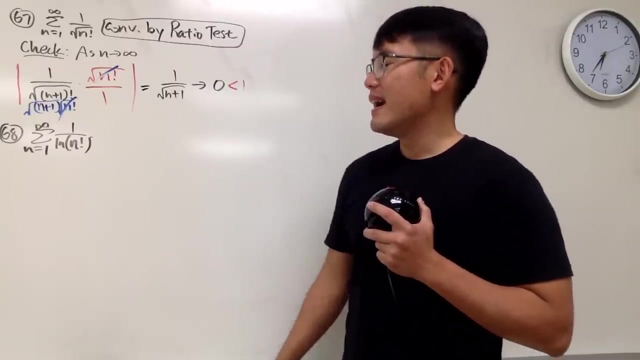 1 over ln n factorial Like this This time, though, Unfortunately, if you do this, They cannot cancel nice d. Okay, they cannot cancel nice d, So Let's see Factorial in the wrong place. This right here actually diverges. Let me show you why. One of the things that you can do: 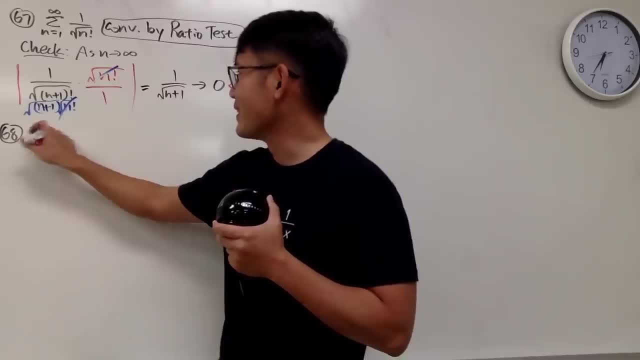 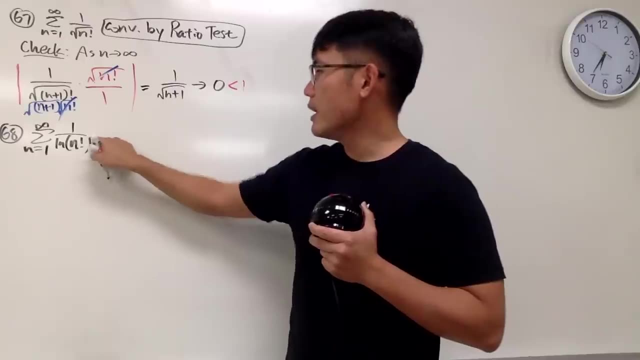 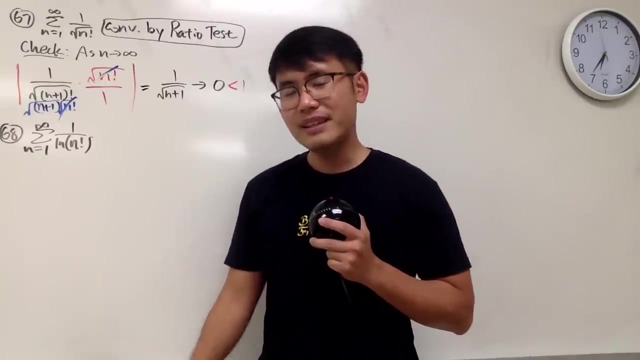 we are putting the factorial into natural log, so sum as n goes from 1 to infinity, 1 over ln, n factorial like this this time, though unfortunately, if you do this they cannot cancel nicely. okay, they cannot cancel nicely. so let's see. 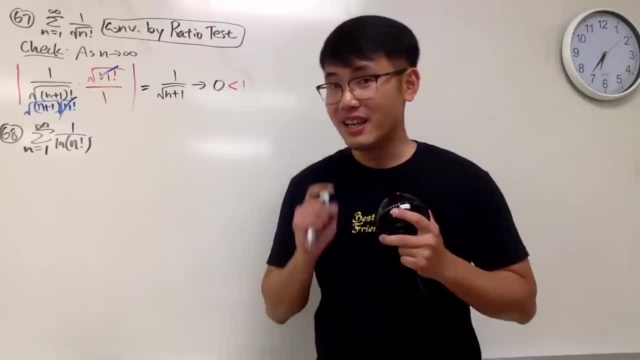 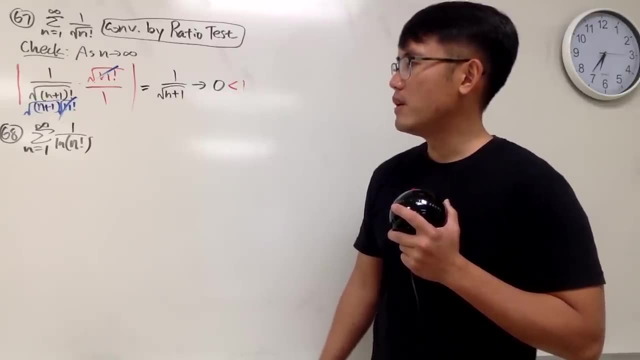 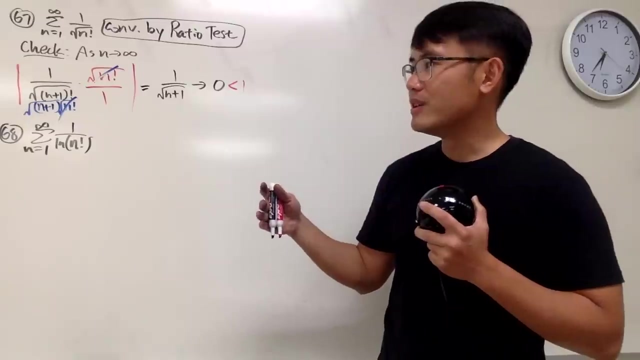 factorial in the wrong place. this right here actually diverges. let me show you why. one of the things that you can do is you can use the definition of the factorial and can, like, break it down into sums and all that. so that's one of the things that we can try. 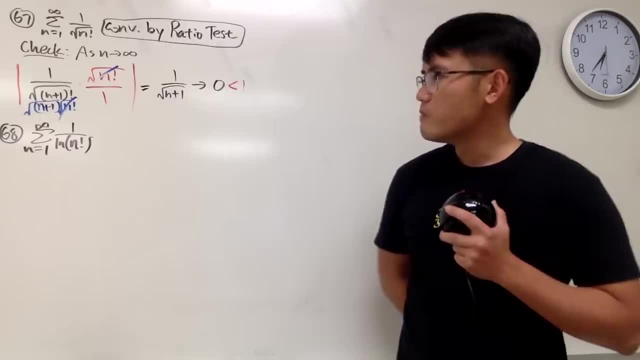 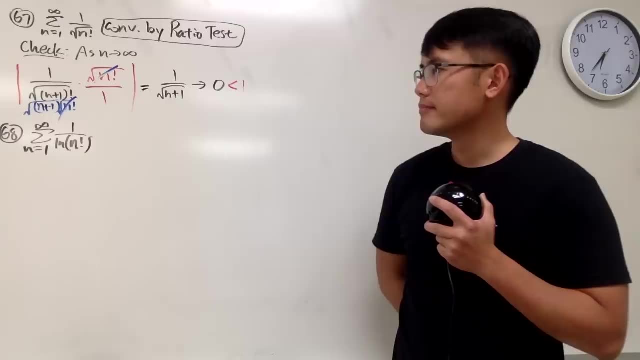 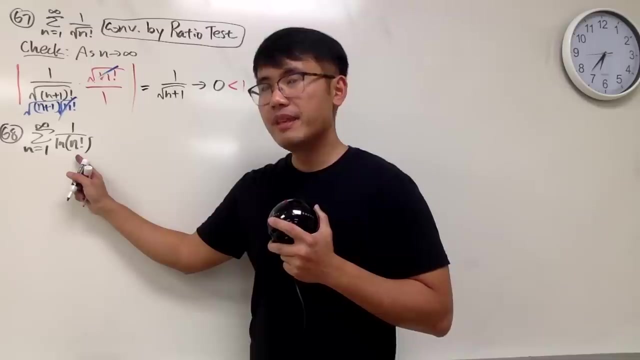 or another way to do this is another ratio test. again, let me tell you what I told you. let's compare with something that we actually did earlier. okay, this right here. so I will just put this down right here for you guys, right. 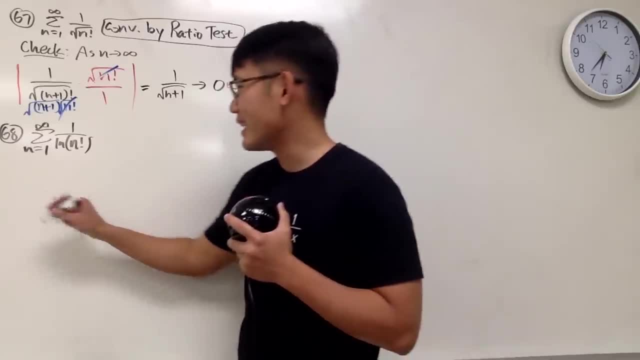 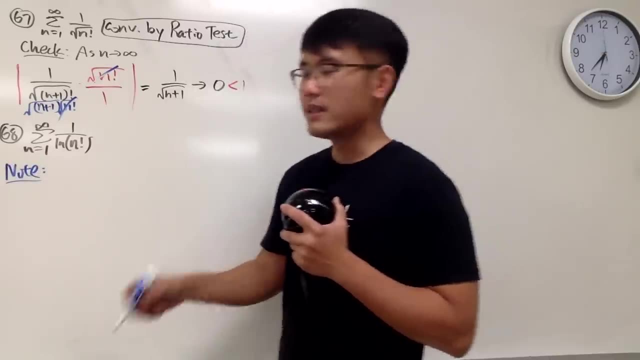 this right here. I can legitimately say it's a recall because we did that. so actually, first of all I'll just say this is a note which is still a note. notice from the list: n- factorial is less than less than n to the n. 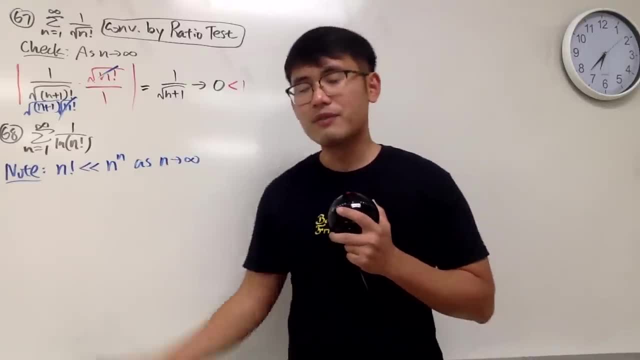 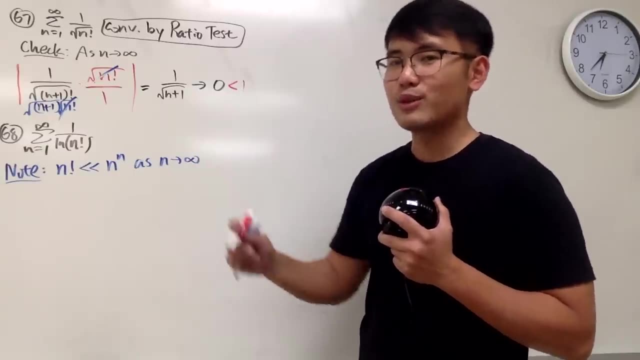 as n goes to infinity. right, that's just from the list. that's why I put on less than, less than, and natural log is an increasing function, so we can just take the natural log from both sides without changing inequality. so when we do that, we have natural log of. 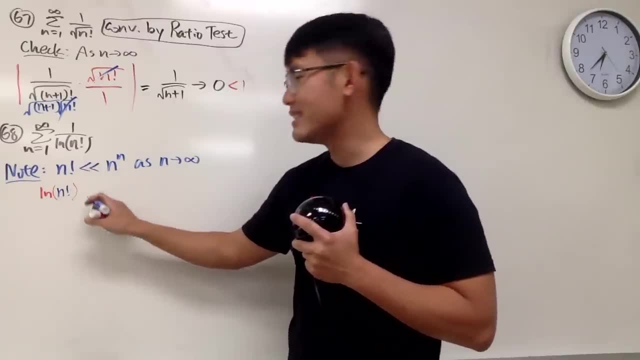 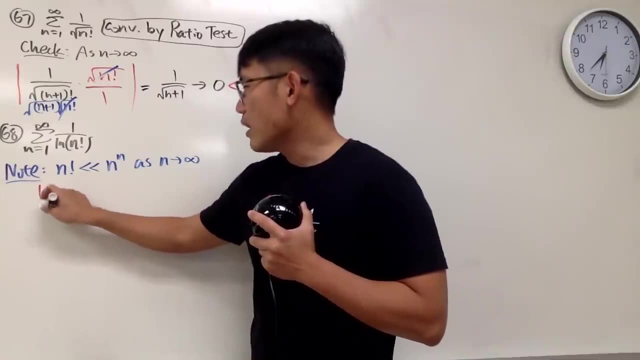 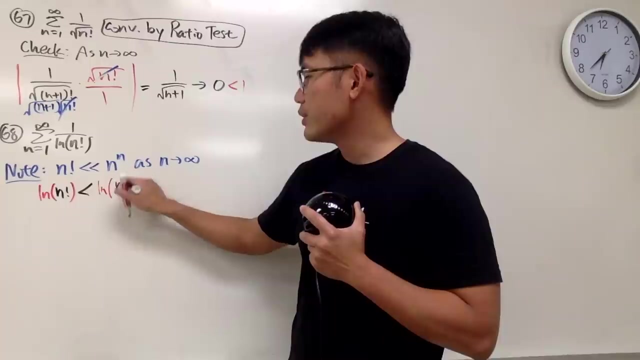 n factorial and let me now just put down one less than right here. actually, now I'll just use black. why am I using black? why am I using blue? okay, natural log of n factorial. this right here will be just less than natural log of n to the n. 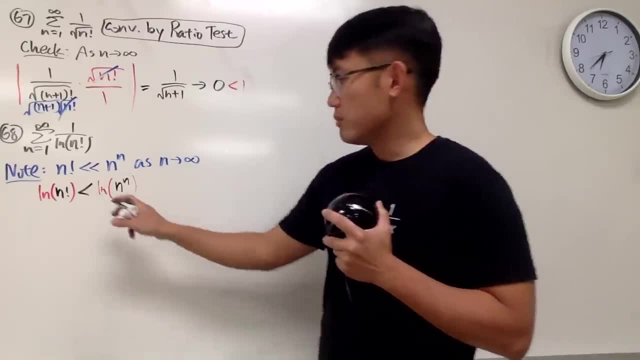 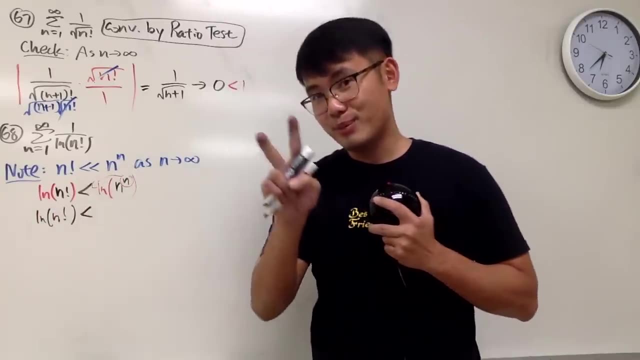 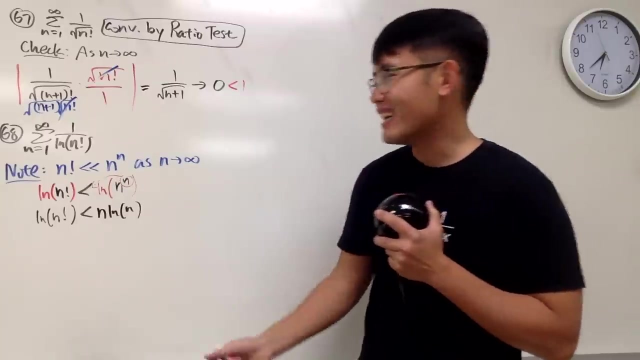 which, if you look at this right here, this is just natural log of n factorial, less than bring the n to the front. that's question number two. isn't it n times natural log of n? and then we can do the reciprocal on both sides? 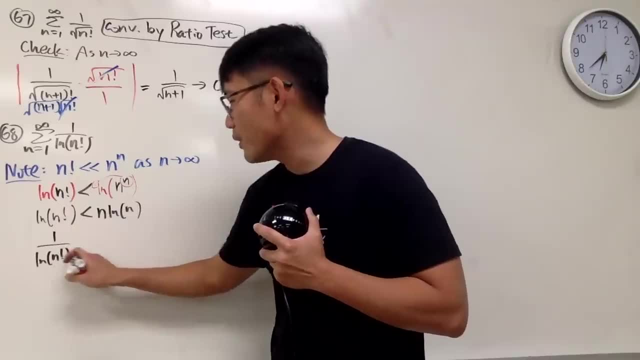 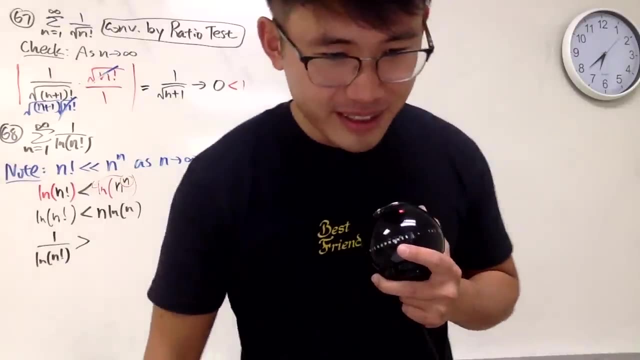 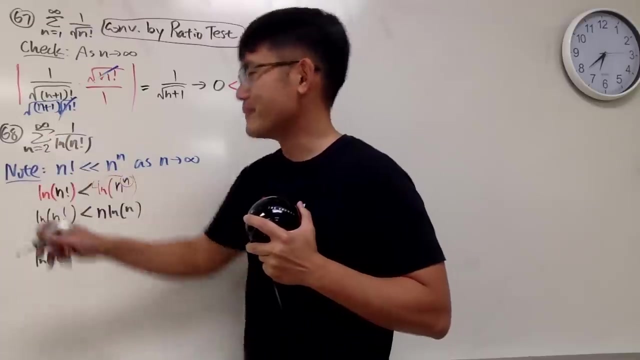 in another word, we get one over natural log of n factorial. it's bigger than again. everything is positive, so we can just do the reciprocal on that. okay, I make a mistake, n cannot be one, okay, ah, okay, okay, okay, sorry, sorry, n has to be start with two, okay. 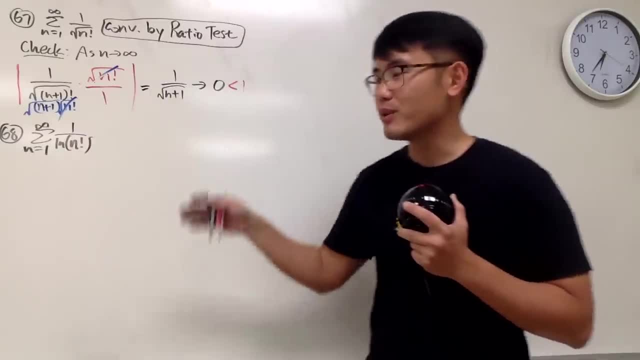 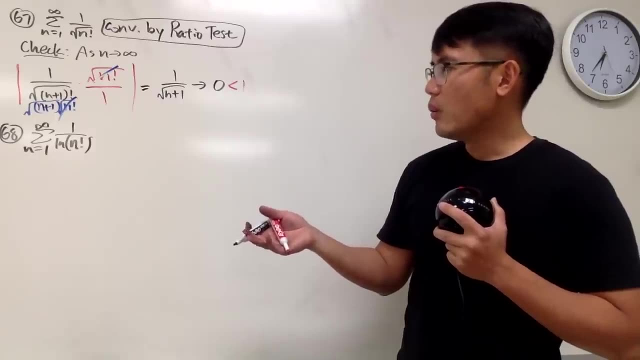 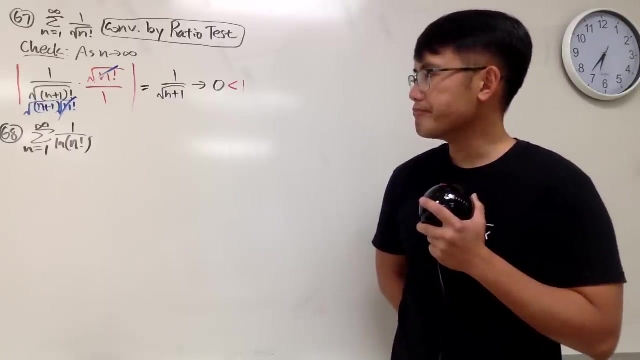 Is you can use the definition of the factorial And can like break it down into sums And all that. So that's one of the things That we can try, Or another way to do this Is Another ratio test. again, As I told you, Let's compare with something. 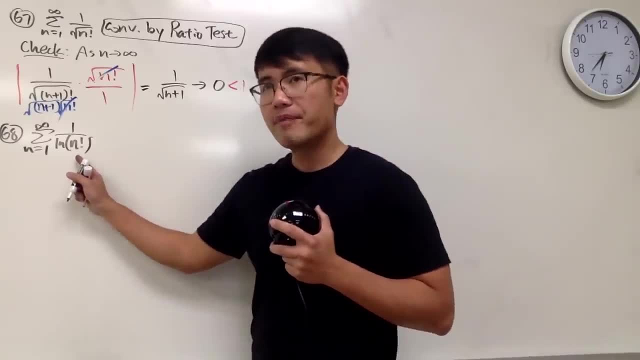 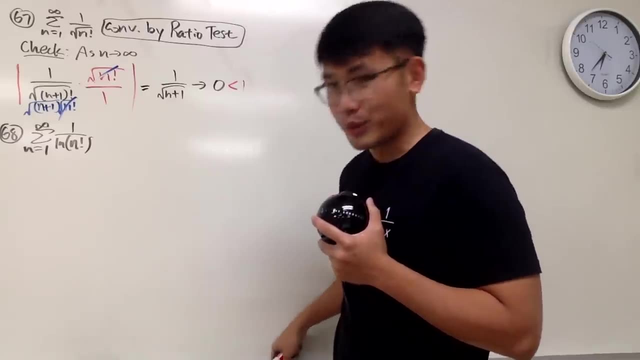 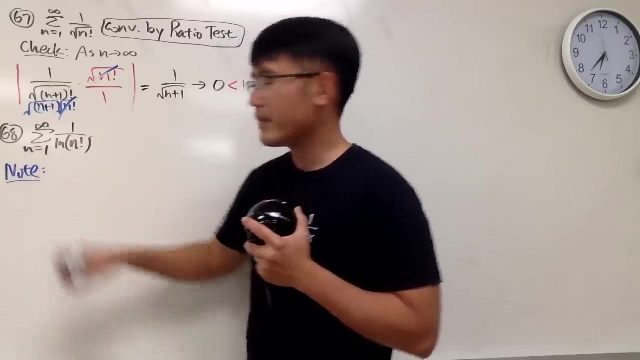 That we actually did earlier. Okay, This right here. I'll just put this down right here for you guys. This right here, I can legitimately say It's a recall, because we did that. So actually, first of all, I'll just say This is a note Notice from the list. 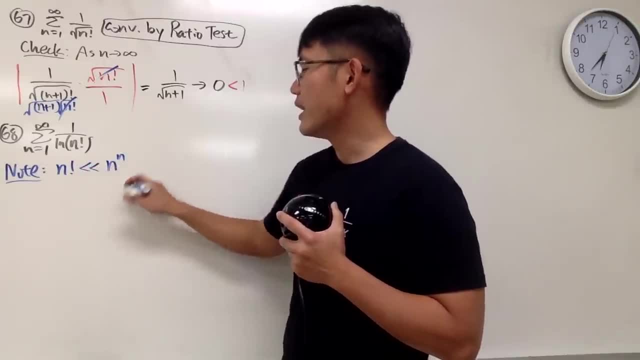 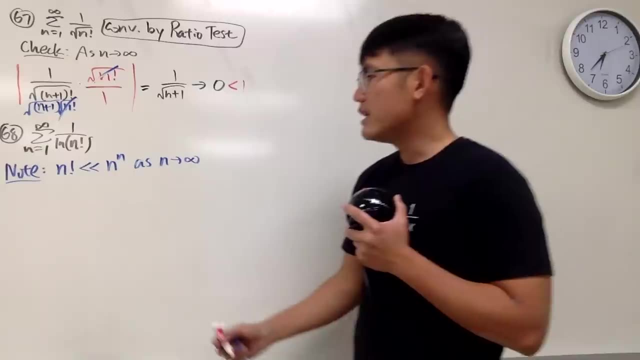 n. factorial is less than less than n to the n, As n goes to infinity. Right, that's just from the list. That's why I put down less than less than. And. Natural log is an increasing function, So we can just take the natural log from both sides. 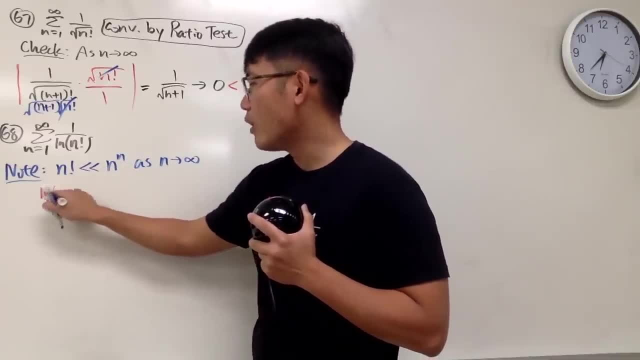 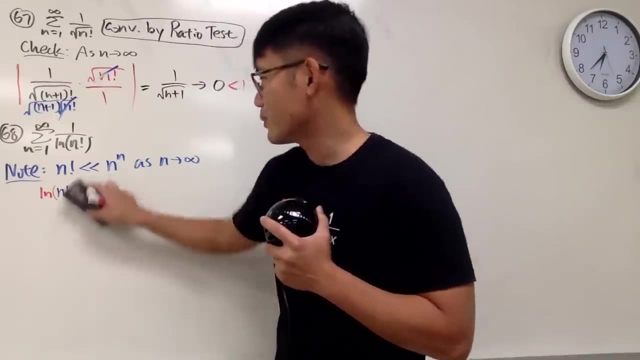 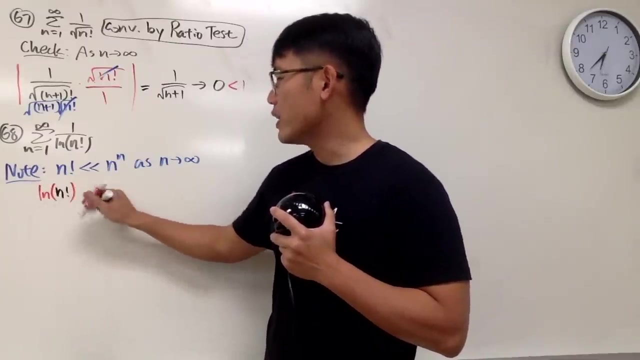 Without changing the inequality. So when we do that, we have natural log of n factorial, And let me now just put down one less than right here. Actually, now I'll just use black. Why am I using blue? Okay, Natural log of n factorial. This right here will be just less than. 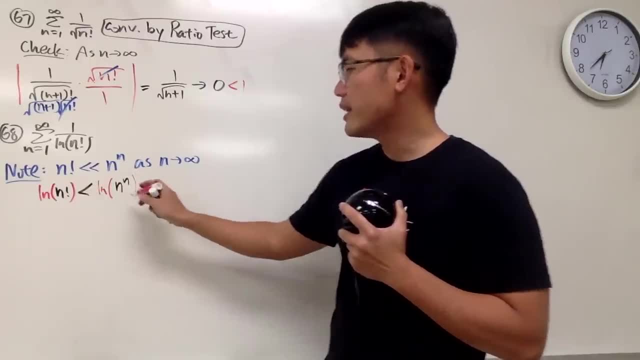 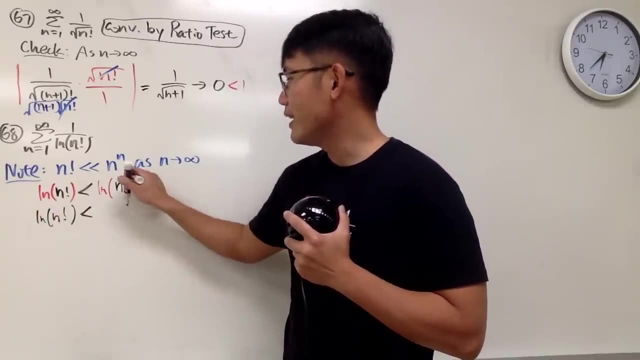 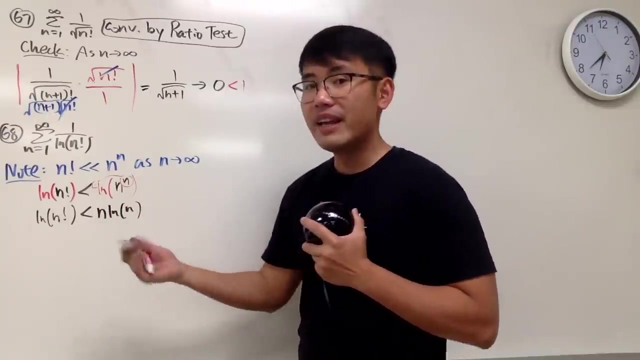 Natural log of n to the n Which, if you look at this right here, This is just natural log of n, factorial, Less than bring the n to the front. That's question number two. Isn't it n times natural log of n? And then we can do the reciprocal on both sides? 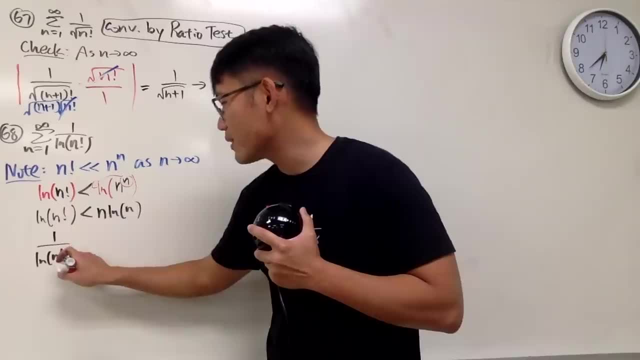 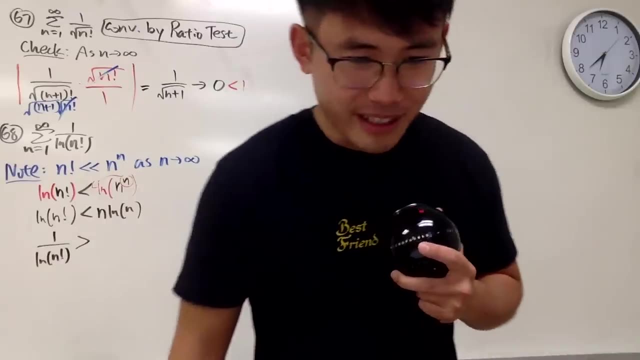 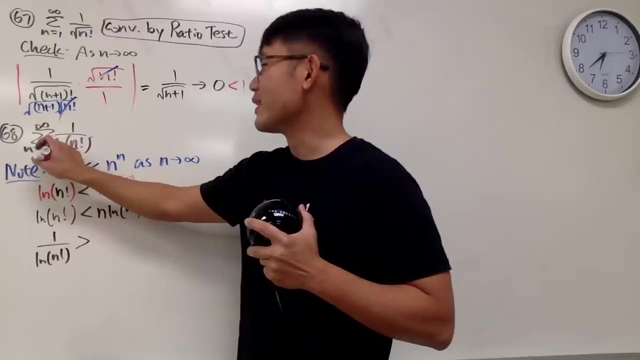 In other words, The natural log of n factorial Is bigger than Again. everything is positive, so we can just do the reciprocal on that. Okay, I make a mistake, n cannot be one. Okay, Sorry, sorry, n has to be starting with two. n has to start with two Because 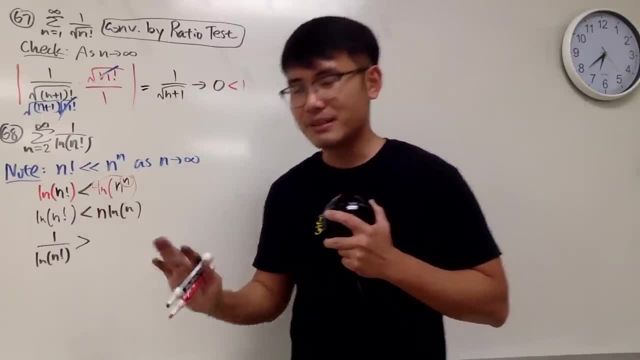 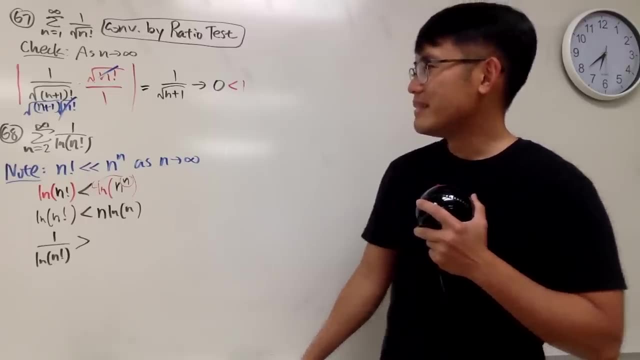 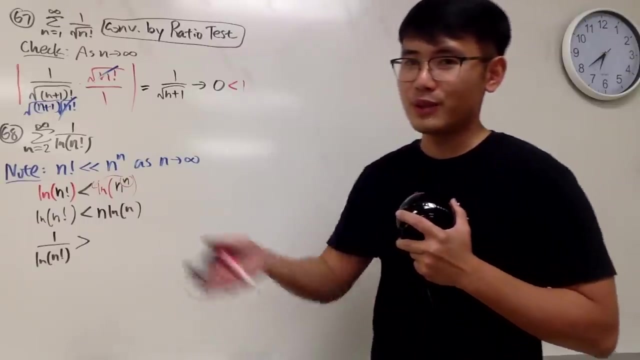 If n is one ln, one is just zero in the denominator. That's all good, That's bad, that's dangerous. Yeah, anyway, Two factorial, Yeah, so this is legit. So this right here. And, by the way, do not change the questions on the final example, So you have to follow it. 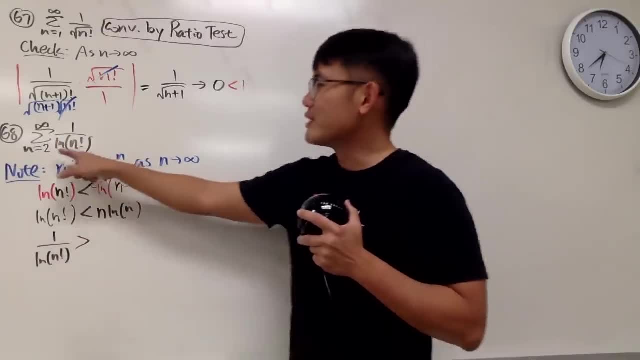 n has to start with two because, yeah, okay, I'll tell you guys. now, if n is one and 1 is just 0 in the denominator, it's all good, right, That's bad, that's dangerous. 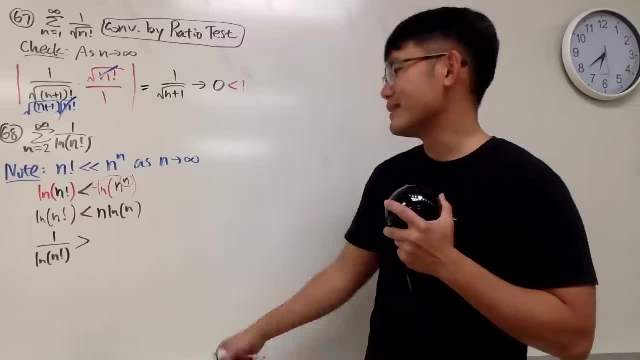 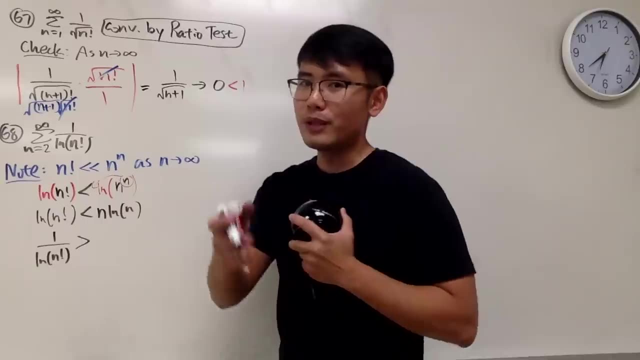 So let's just put down 2 for that. Yeah, Anyway, 2 factorial 2, yeah, so this is legit. So this right here. and, by the way, do not change the questions on the final example. so you have to follow it. 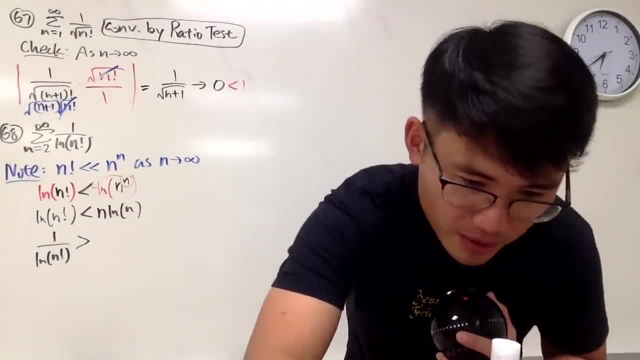 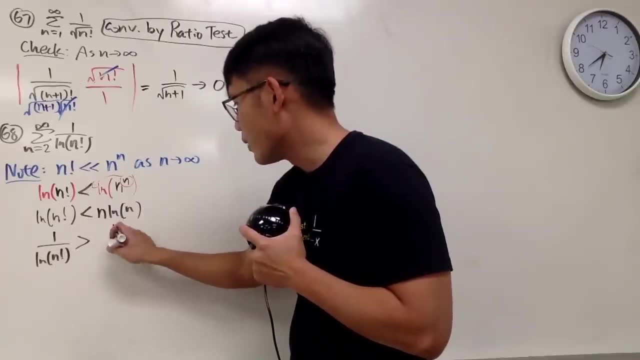 This is just my mistake on the title, so now I'll change it so it should be 12.. I'll fix it for the PDF for you guys, All right? anyway, do the reciprocal on both sides. This is 1 over n, ln, n like this: 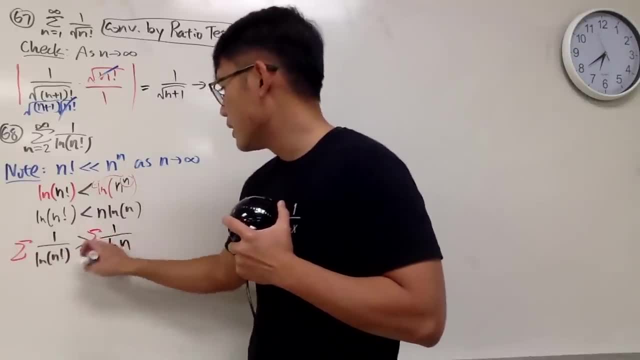 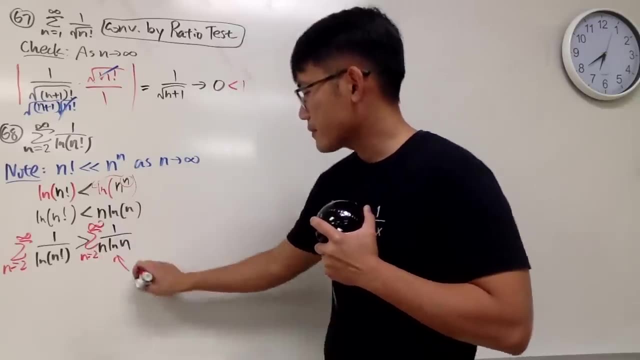 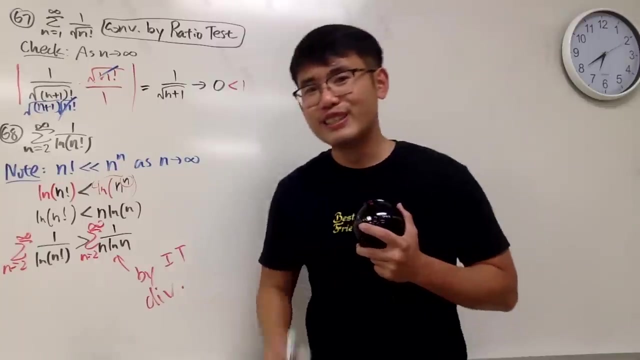 And now, of course, if you look at the series as n, going from 2 to infinity, we did this by the integral test. We did that. this right here diverges. So, in other words, this right here also diverges. 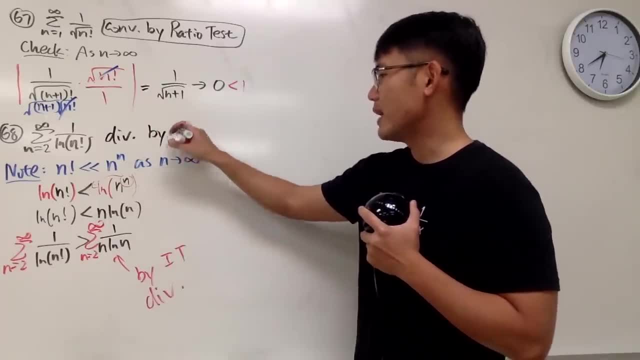 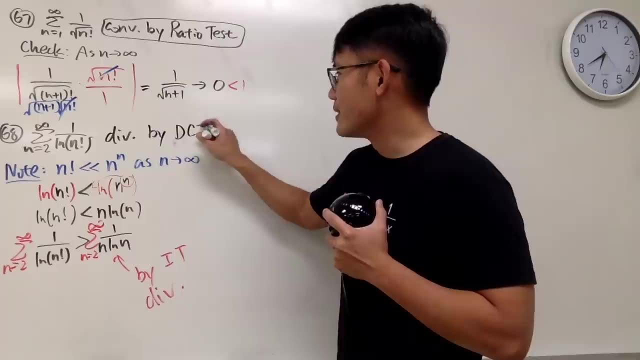 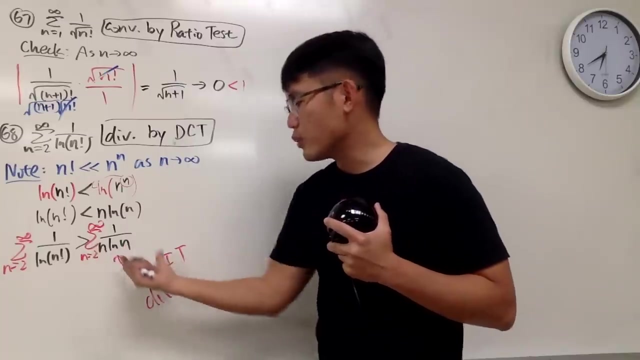 by technically comparison right. And I'll say: this is the direct, this is not the O, this is the direct comparison test. All right, And if you are doing this from scratch, then of course you have to provide the integral test on your own. 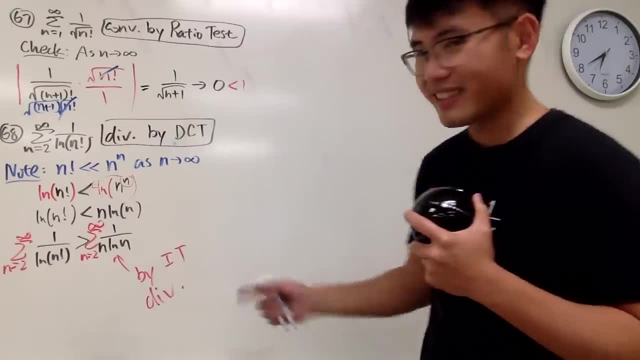 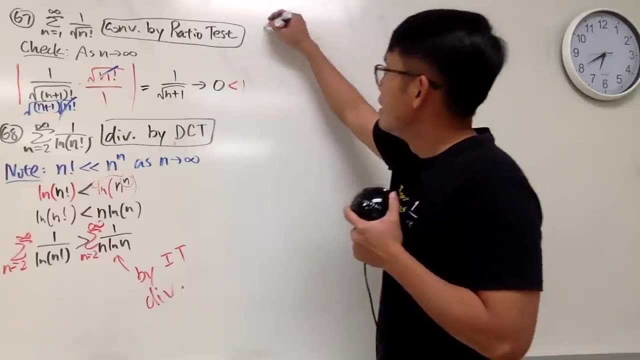 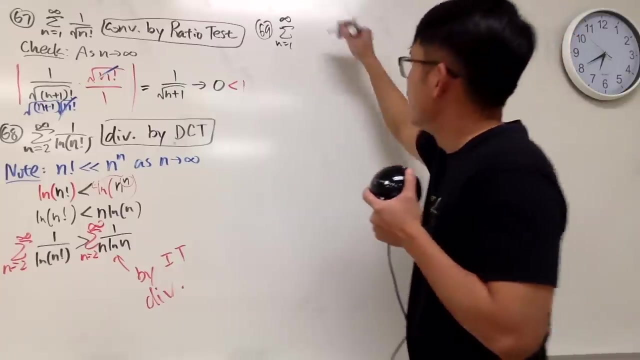 but this is question number 2.. We did that already, so go check that out. Very cool. Now number 69.. The sum as n goes from 1 to infinity: n okay, n n plus 2, parentheses and all that. 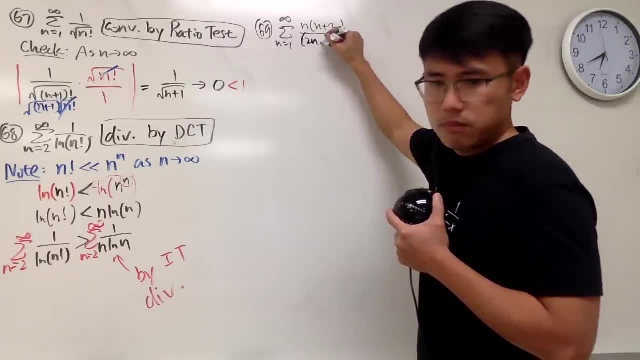 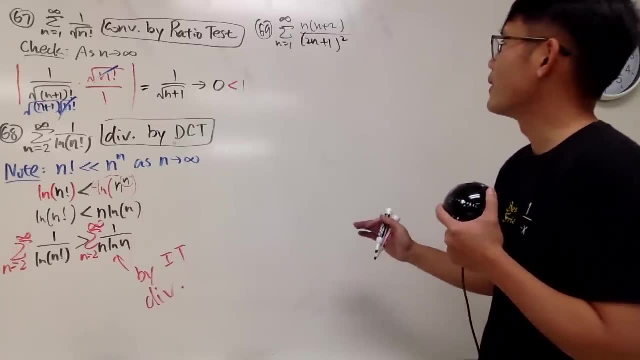 and then we have 2n plus 1 squared, like all this. Well, this is very. this is not so bad. It's just like power functions and all that. But the problem is that on the top notice we have n squared. 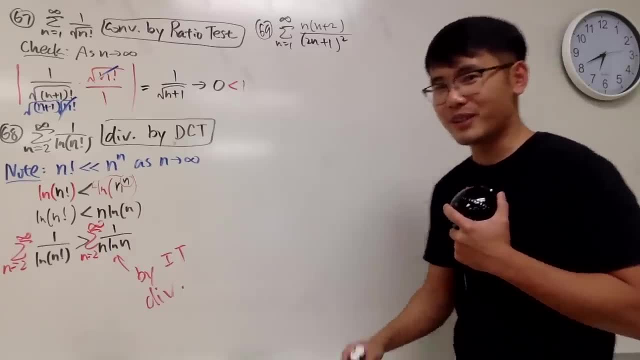 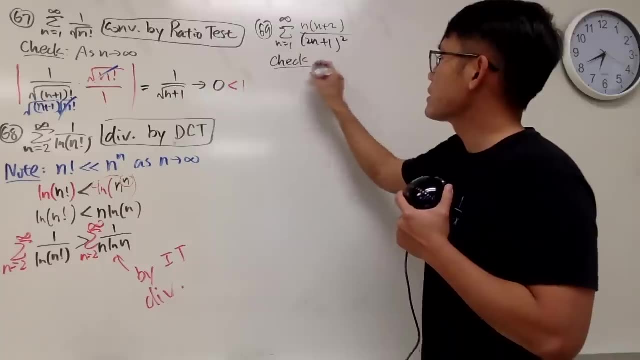 On the bottom we also have the n squared term. Don't trick us, okay, Don't trick us for this question, Don't be triggered on this as well. So test for divergence, We will check. We will check the limit as n goes to infinity. 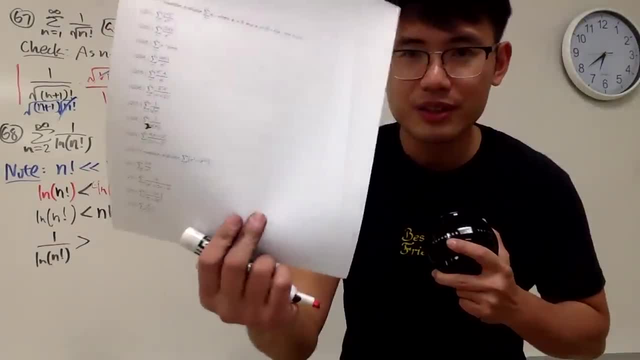 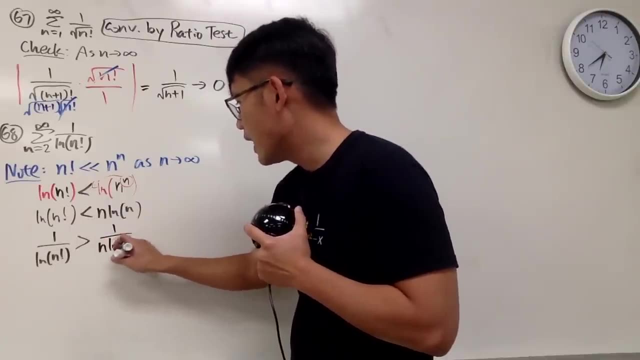 This is just my mistake on the On the title, So now I'll change it. I'll fix it for the PDF for you guys, Alright, anyway, do the reciprocal on both sides. This is one over n ln n Like this. And now, of course, if you look at the series, 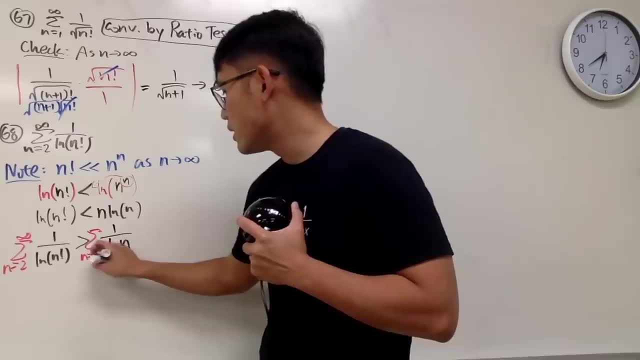 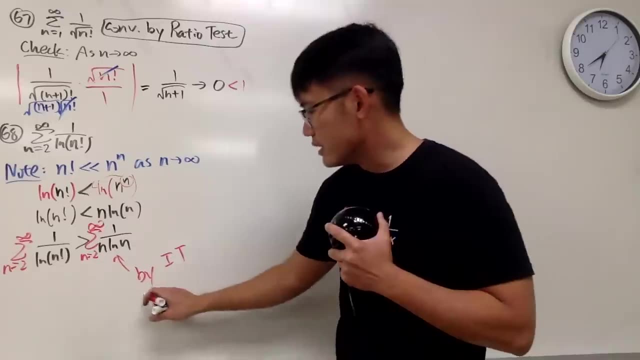 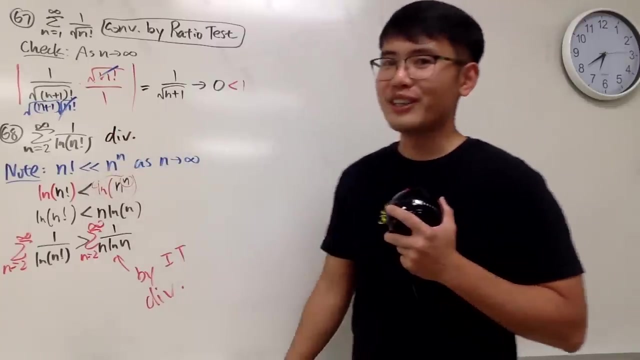 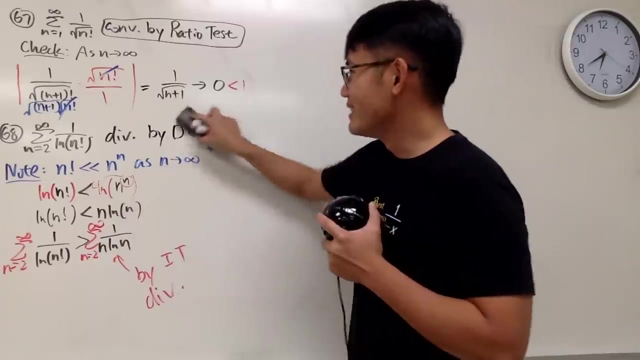 As n, going from two To infinity. We did this By the integral test, We did that. This right here Diverges. So, in other words, This right here also diverges By technically comparison. Okay, And I'll say: this is the direct, This is not the all, This is the direct. 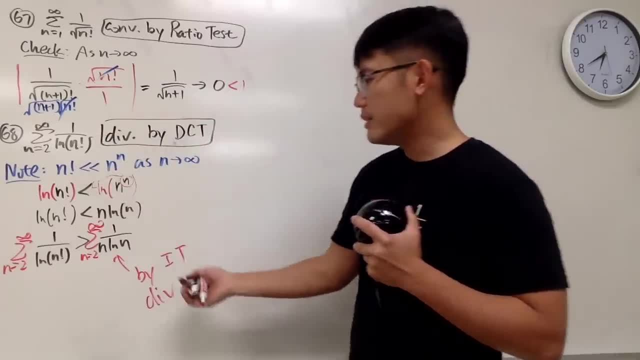 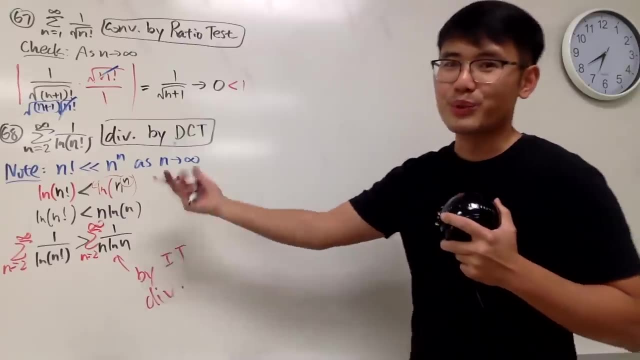 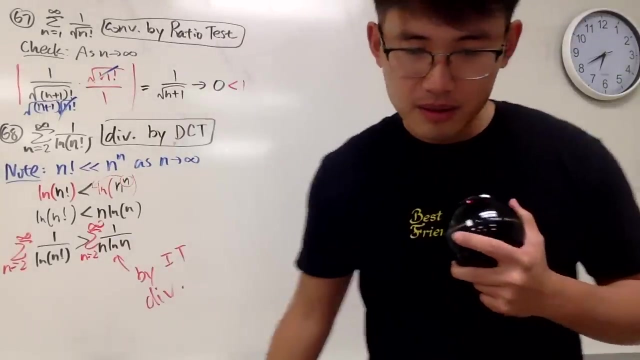 Direct comparison test. Okay, So if you are doing this from scratch, Then of course you have to provide the integral test On your own. But this is question number two. We did that already, So go check that out. Very cool. Now number 69: The sum As n goes from one. 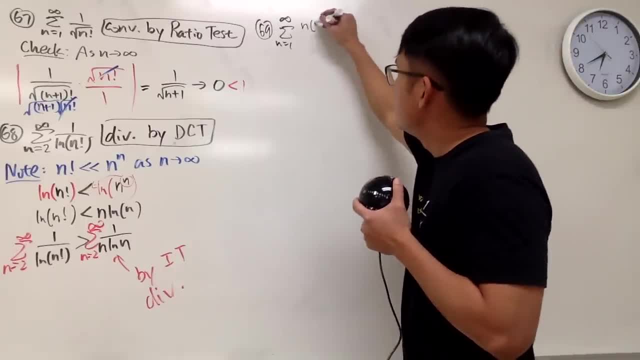 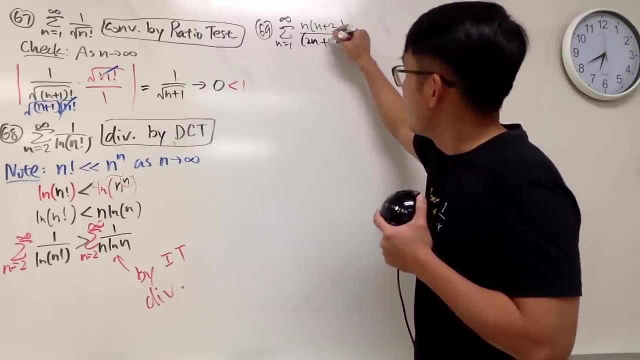 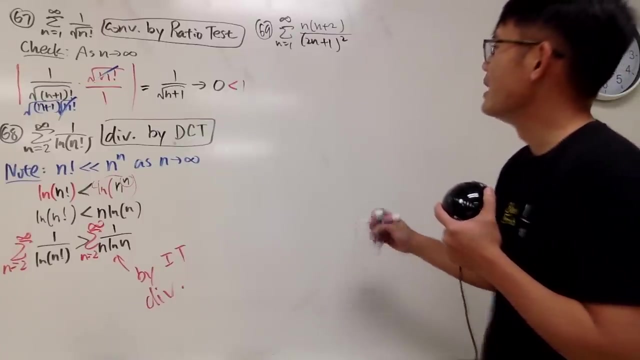 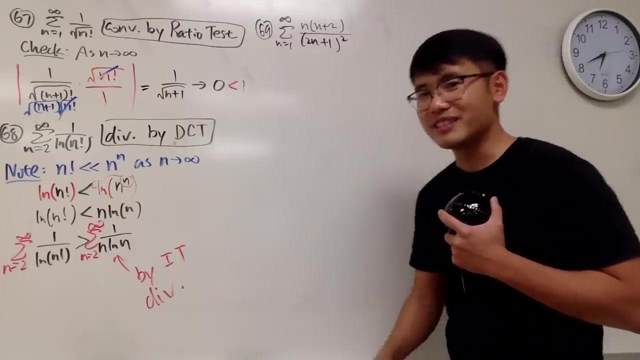 To infinity. N, Okay, n, N, plus two Parentheses, and all that Plus one Square like all this. Well, this is very. This is not so bad, It's just like power functions and all that. But the problem is that On the top notice, we have n squared. On the bottom, we also have the n squared term. 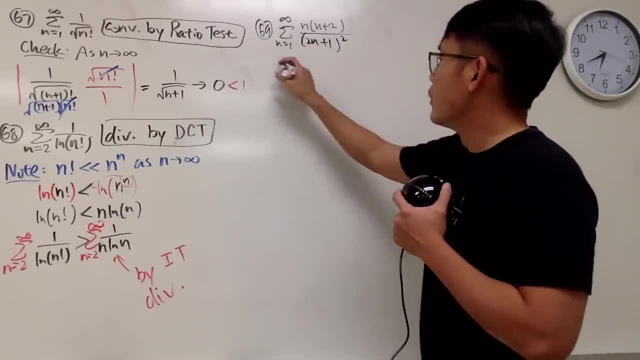 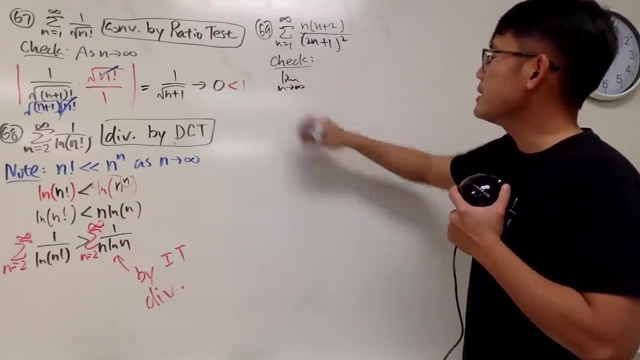 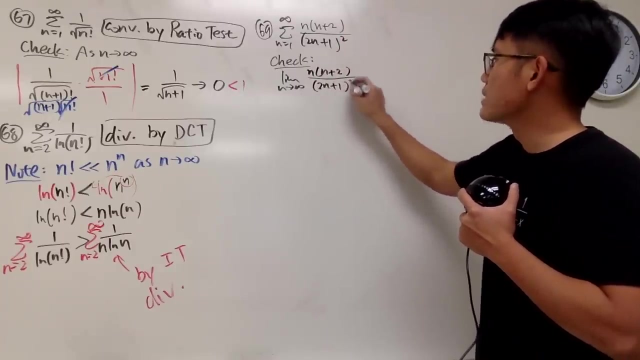 Don't trick us, okay, Don't trick us for this question, Don't be tricky on this as well. Test for divergence: We will check the limit As n goes to infinity, And I will just put this down: n times n plus two, Over parenthesis, two n plus one. 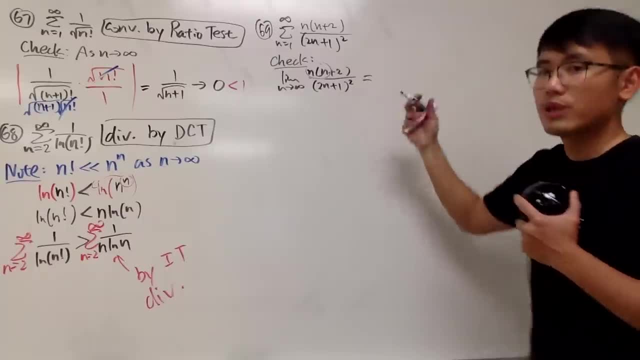 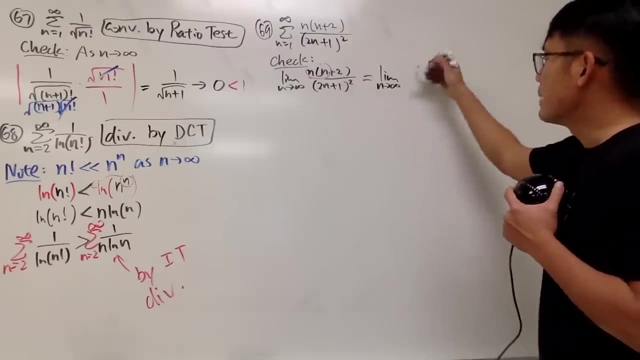 Square. Well, on the top, you see, we care about this, Which is just going to give us n squared. So this is just the limit, As n approaching infinity. On the top is pretty much just n squared And on the bottom, Don't forget, you have to just pair this up. 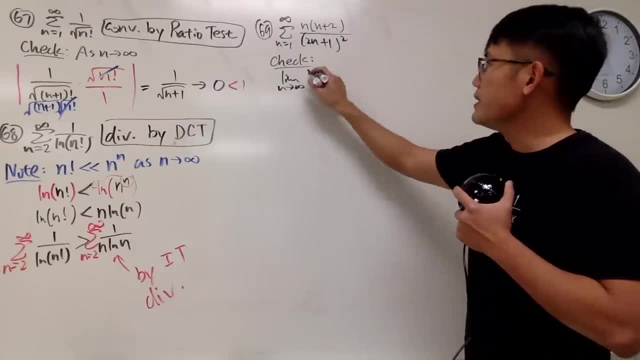 right here: limit and we'll check the limit And I will just put this down: n times: n plus 2 over parentheses, 2n plus 1 squared. Well, on the top you see, we care about this- which is just going to give us n squared. 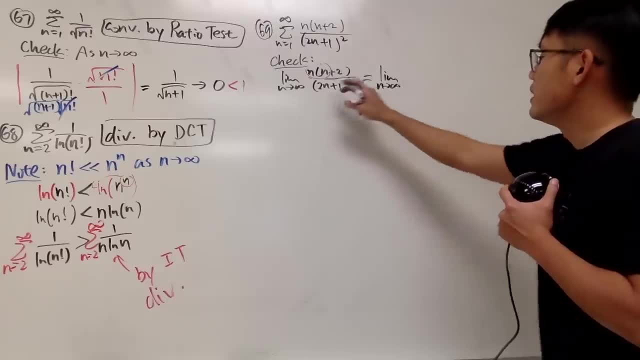 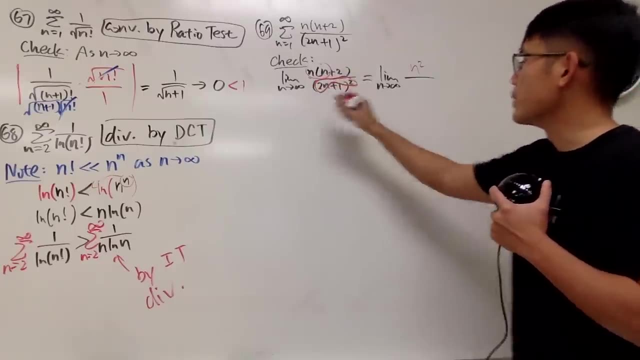 So this is just the limit as n approaching infinity. On the top it's pretty much just n squared, And on the bottom- don't forget- you have to just pair this up So we get 4n squared. All in all, the limit that we end up with is just 1 over 4,. 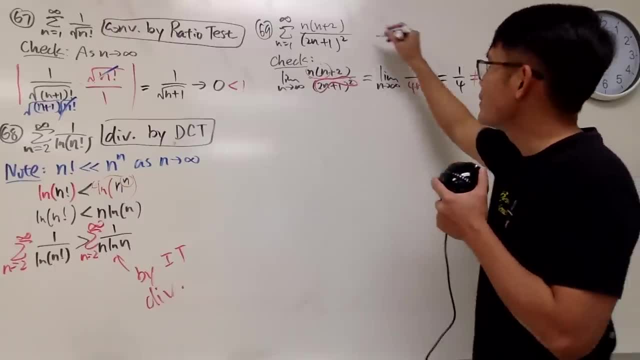 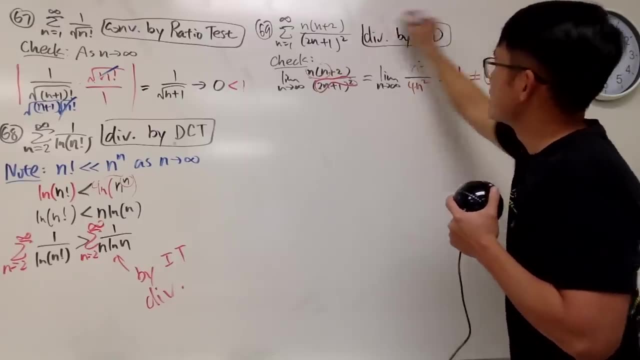 which is not 0.. Therefore, this is test for divergence. This right here. Divergence by t of d: Very, very nice. Okay, now 30 more to go. Oh my God, 30 more to go. 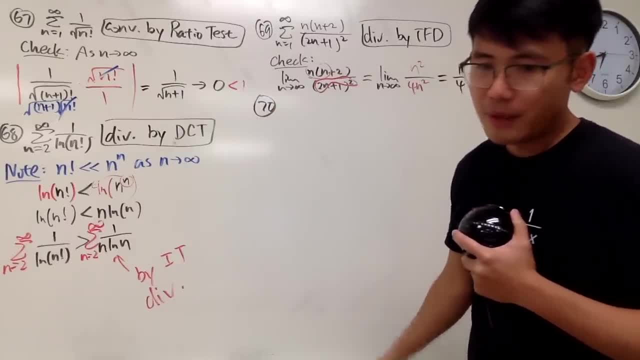 Number 70.. If possible, evaluate the sum as n goes from 1 to infinity. Number 70.. If possible, evaluate the sum as n goes from 1 to infinity. Number 70.. If possible, evaluate the sum as n goes from 1 to infinity. 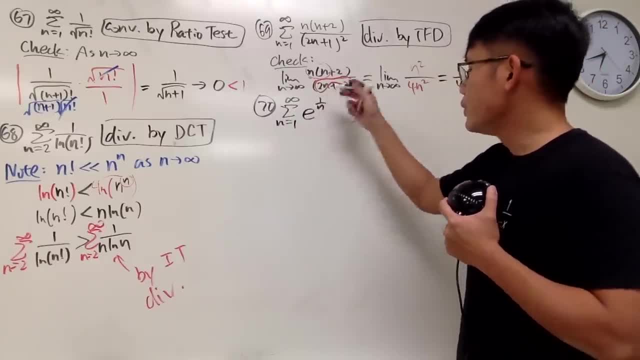 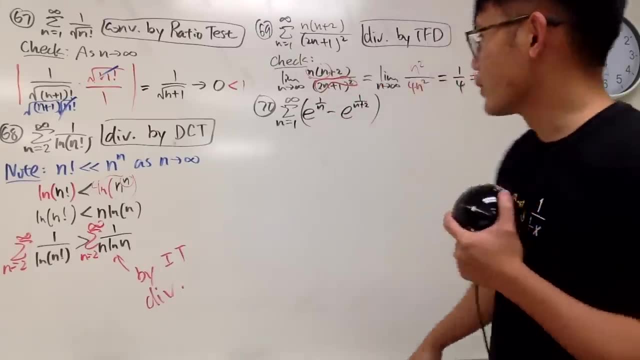 And we have e to the n, e to the 1 over n minus, e to the 1 over n plus 2.. Like this: Now let me show you guys the quick way to do this. Well, actually, now let me just still show you guys all the details, okay. 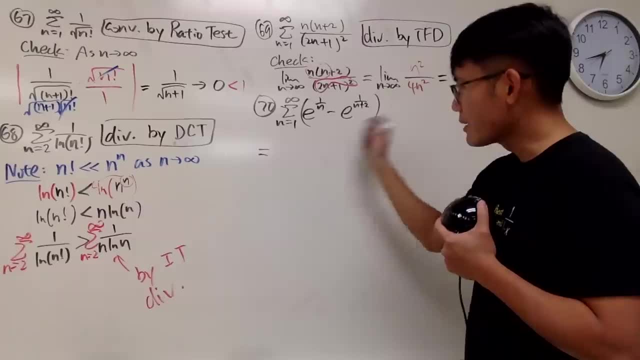 So just write down all the things that you have to do. So plugging 1,, plugging 2, and all that. So let's go ahead and do that. First 1 over 1,, right, And then minus e to the 1 over 3.. 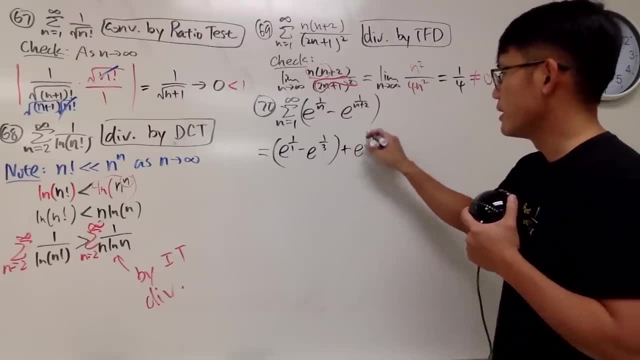 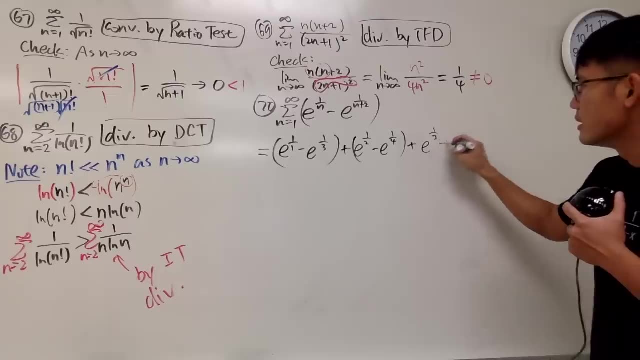 You know the deal. This is going to be telescopic And I'll tell you guys the secret at the end. So 1 half minus 1 over 4 for the new powers Next, e to the 1 third, minus e to the 1 fifth. 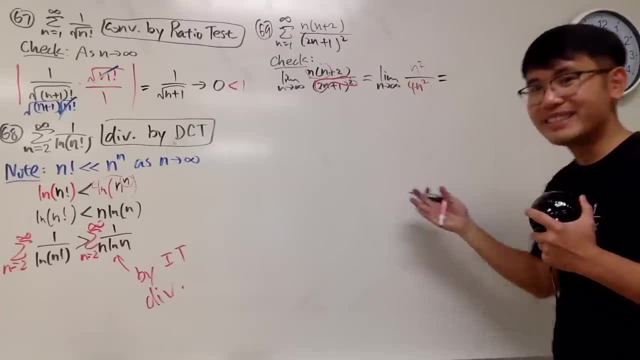 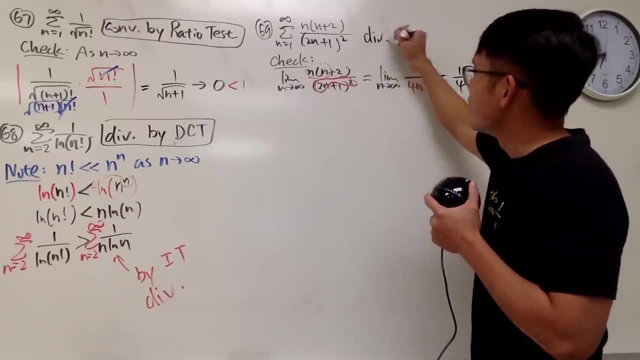 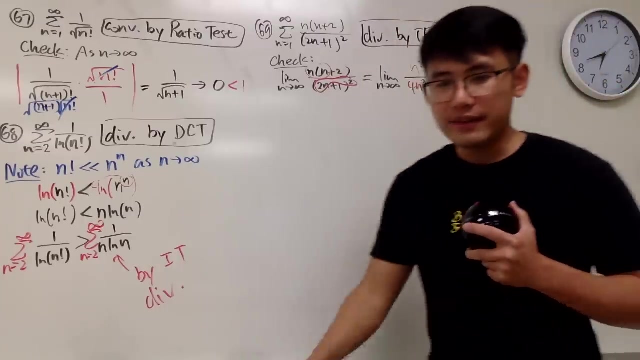 So we get four n squared. All in all, The limit that we end up with is just one over four, Which is not zero. Therefore, this is test for divergence. This right here, Divergence By t of d, Very, very nice. Okay, now thirty more to go. Oh my god. 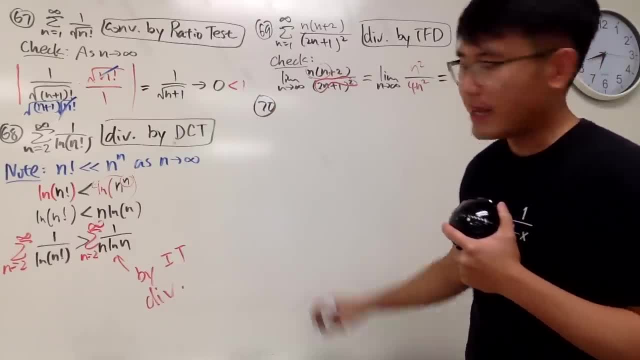 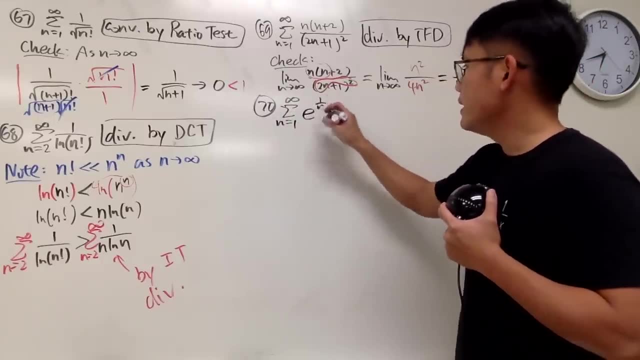 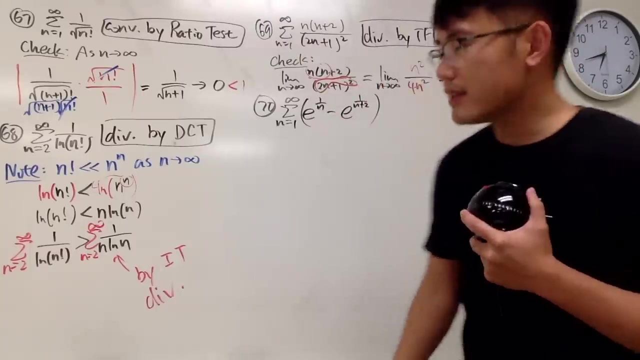 Thirty more to go. Number seventy, If possible, evaluate the sum As n goes from one to infinity And we have e to the n, e to the one over n Minus e to the one over Two, like this. Now let me show you, guys, the quick way To do this. 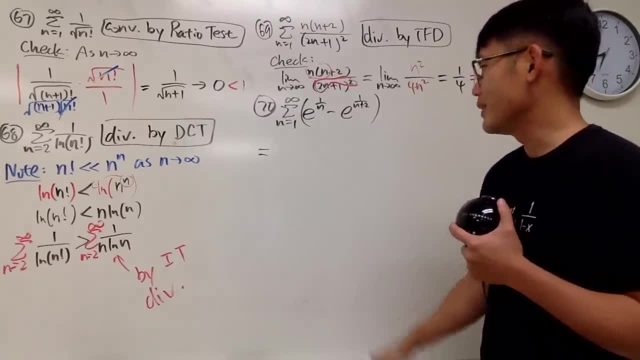 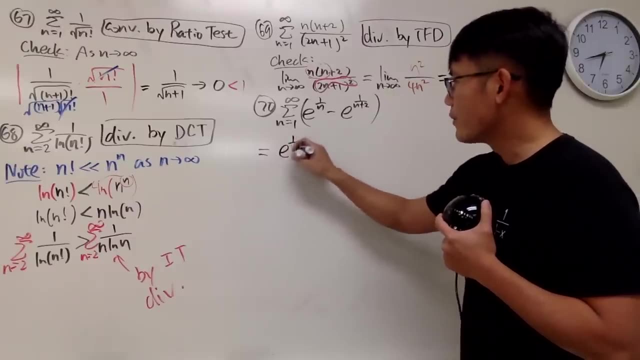 Well, actually now let me just Show you guys all the details. Okay, so just write down all the Things that you have to do. So plug in one, plug in two and all that. So let's go ahead and do that, First one over one, and then minus e to the one over three. 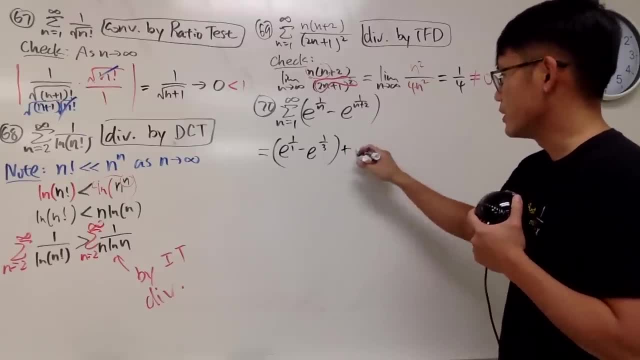 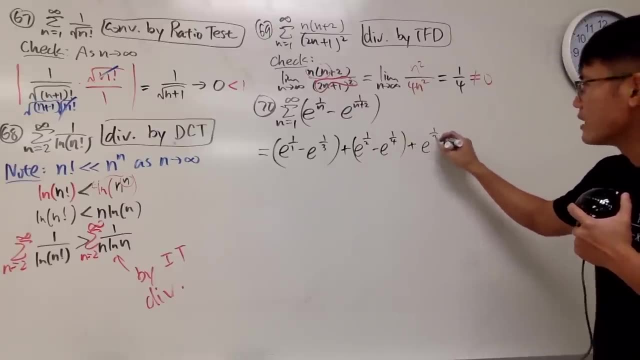 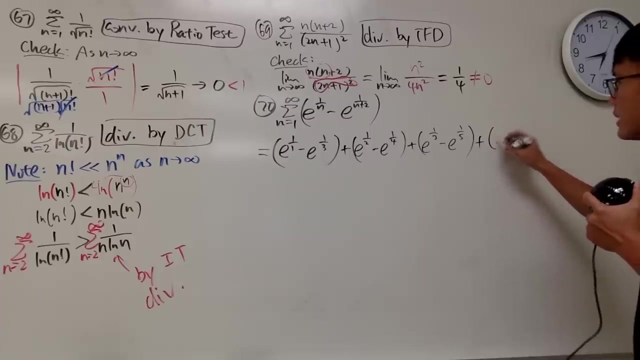 You know the deal. This is going to be telescoping And I'll tell you guys the secret at the end. So one half minus one over four For the new powers, One third minus E to the one fifth, And then next And just do E to the one fourth. 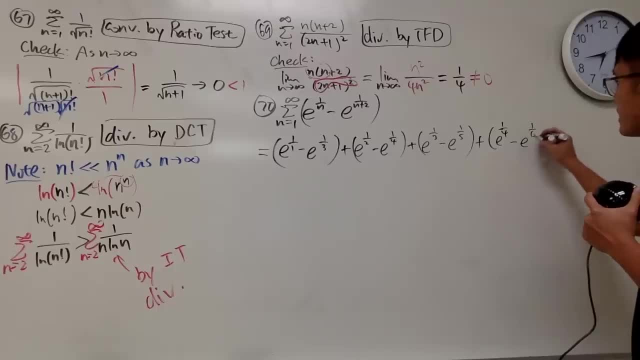 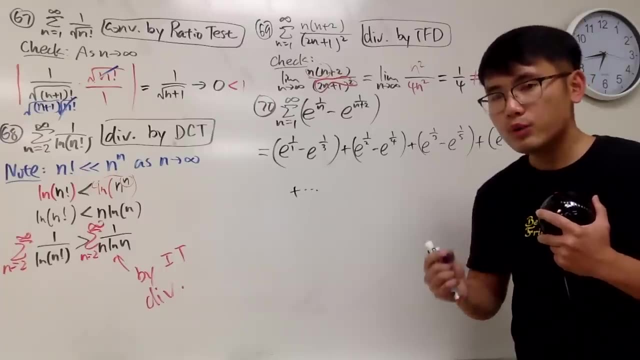 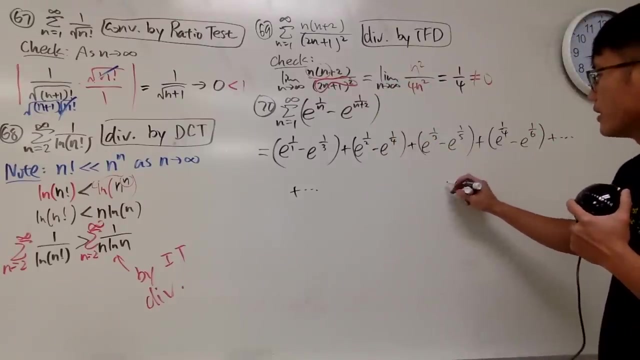 Minus e to the One over six, And so on, so on. so on, Right, And remember We have to write down The nth term. So we have to write down this right here. So I will actually write it down Somewhere here. this is the nth term, Plus e to the one over n. 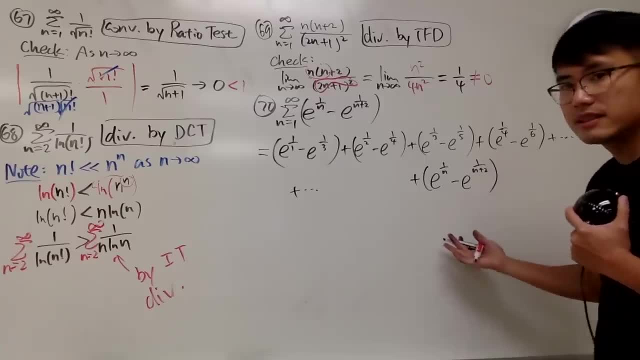 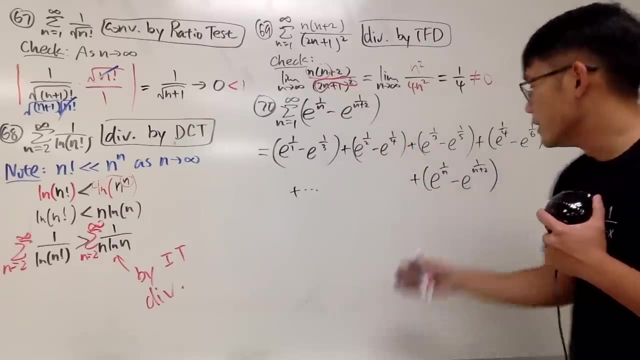 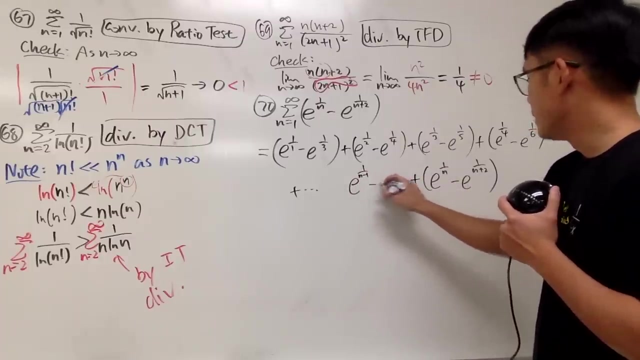 Minus e to the one over n plus two, Like this In this case: Notice the Notice the n and n plus two, It's all by two. So be sure you write down this And then the term before it. So I will also write down E to the one over n minus one. 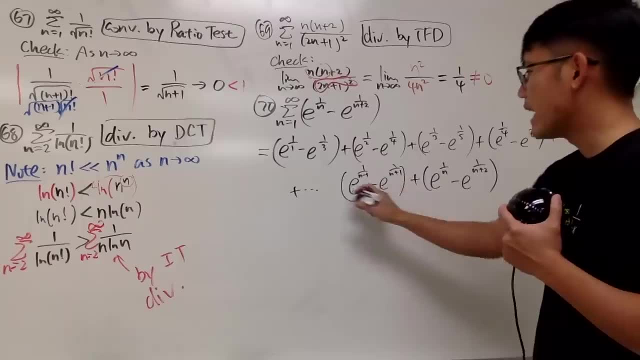 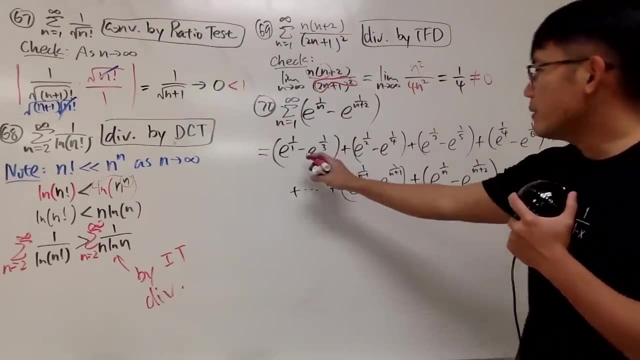 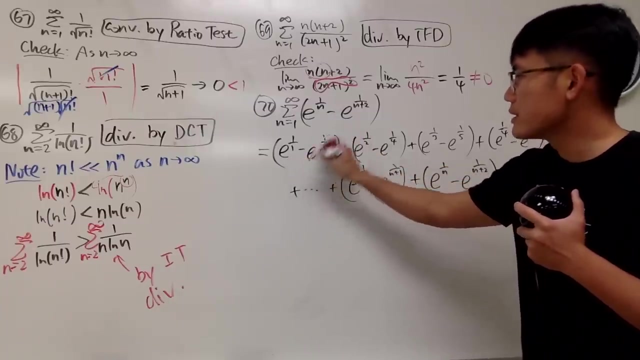 Minus. e to the one over. n plus two. This is the n minus one term And again you write this down Now And all that. check this out Here. This is the reason why you write down by two: This stays negative. e to the one third. This will be cancelled out. 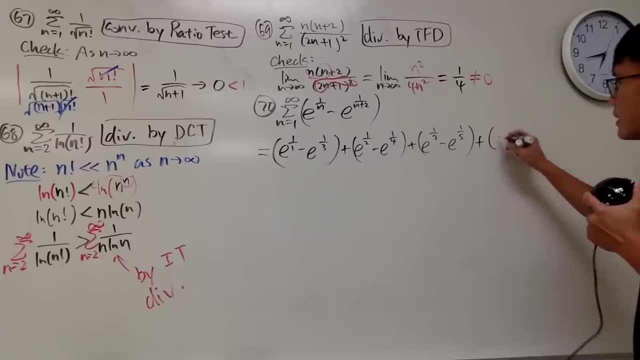 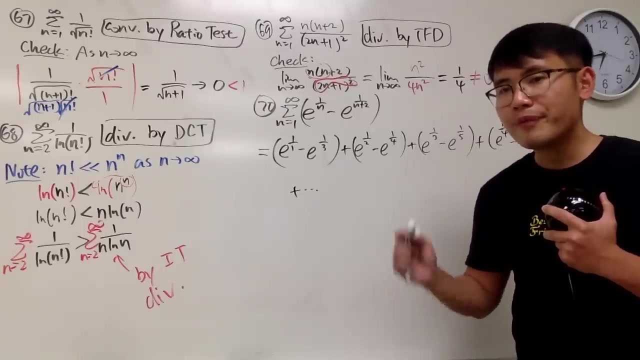 And then next, and just do e to the 1 fourth minus e to the 1 over 6. And so on, so on. so on, right, And remember we have to write down the n star, So we have to write down this right here. 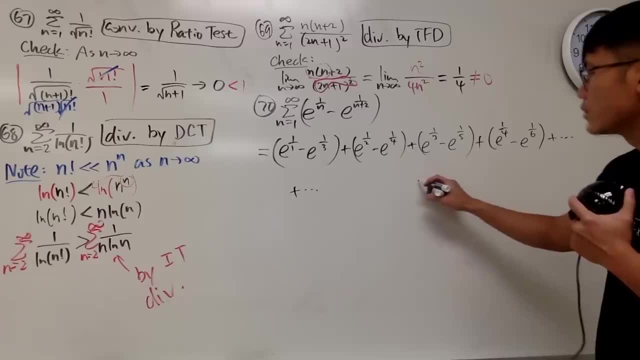 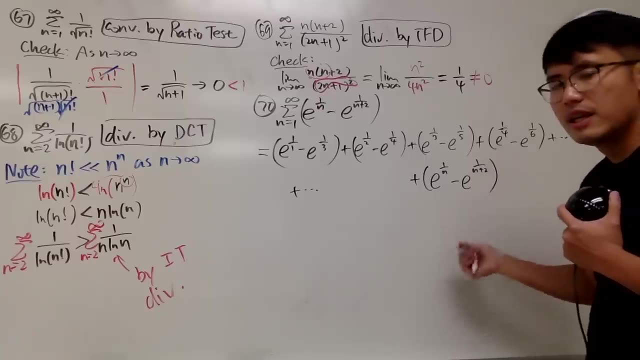 So I will actually write it down somewhere here. This is the nth term, So I will just put down: plus e to the 1 over n, minus e to the 1 over n plus 2.. Like this: In this case, notice the n and n plus 2.. 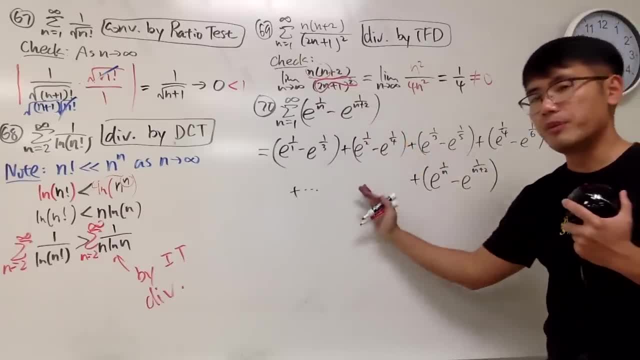 It's all by 2.. So be sure you write down this and then the term before it. So I will also write down e to the 1 over n minus 1 minus, e to the 1 over n plus 2.. 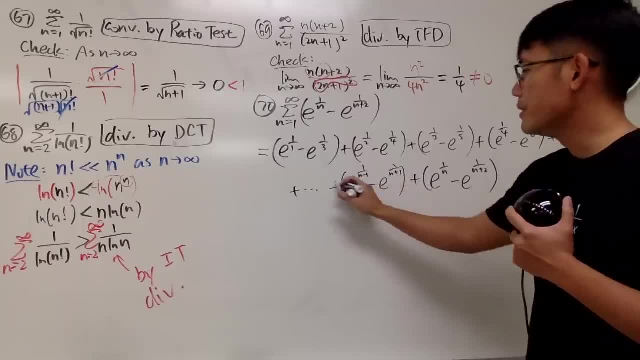 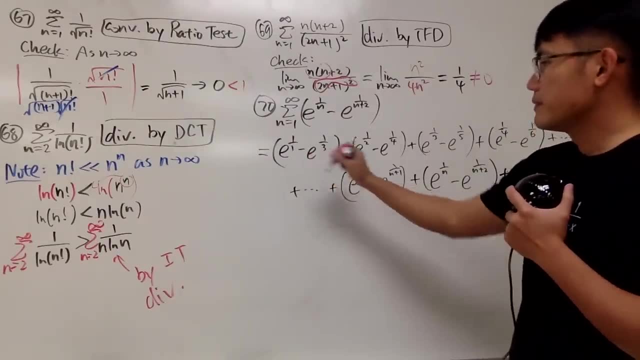 This is the n minus 1 term And again you write this down because you have this being off by 2.. Now, da, da, da and all that. Check this out Here. this is the reason why you write down by 2.. 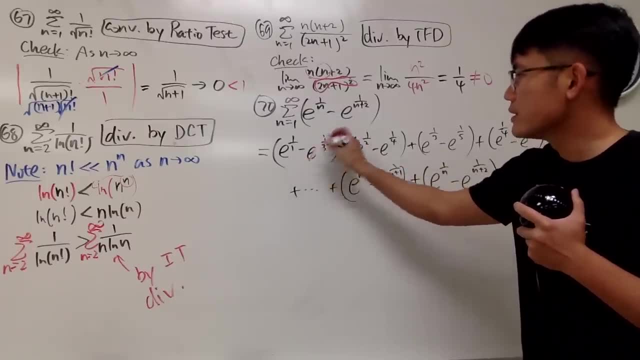 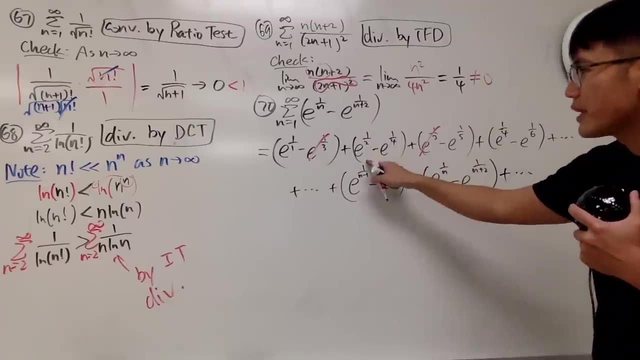 This stays Negative. e to the 1 third. This will be cancelled out. Not this, not this, but this Right. This is like a jump: This right here stays, This right here, cancelled out with that. Okay. So notice: this right here will also be cancelled out with something after this right here. 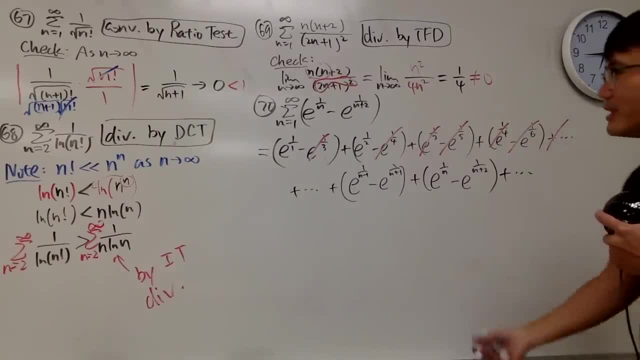 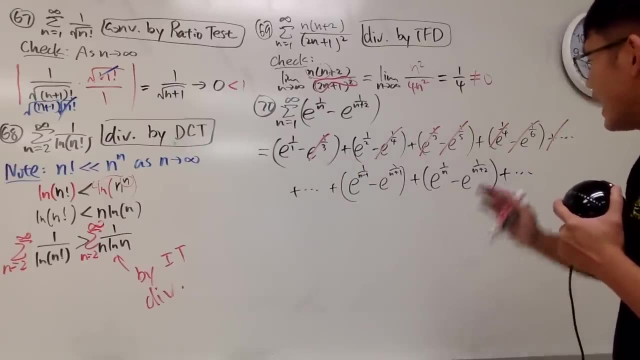 Right, And this right here will be cancelled out with something after that, And the truth is, you will have two terms remained, Right. Two terms remained, And you also have the following: Somewhere right here: Right, Somewhere right here. 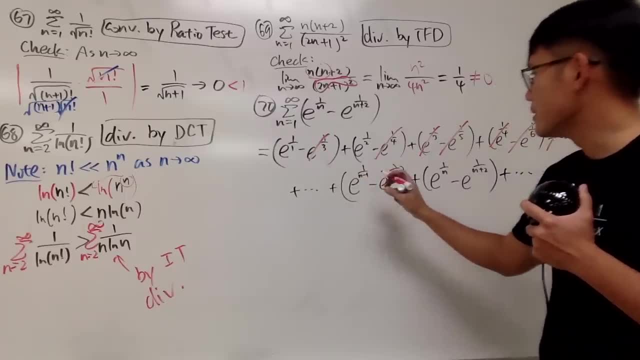 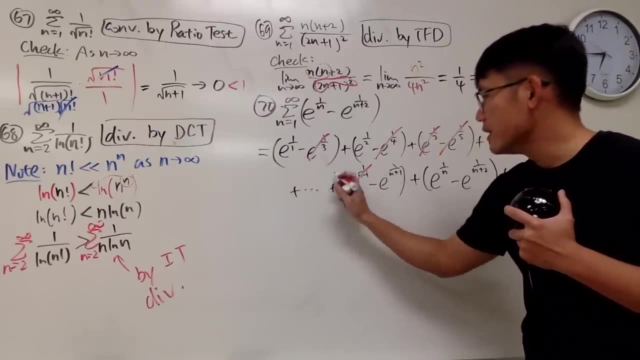 Somewhere right here. actually, We will cancel out this guy. first, Let me see: Yeah, somewhere in the front it's going to have something that cancels out. It's this, And then the term right before this: this guy. it's going to cancel out with this guy. 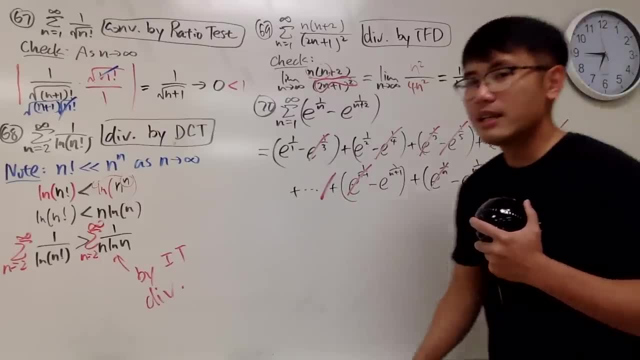 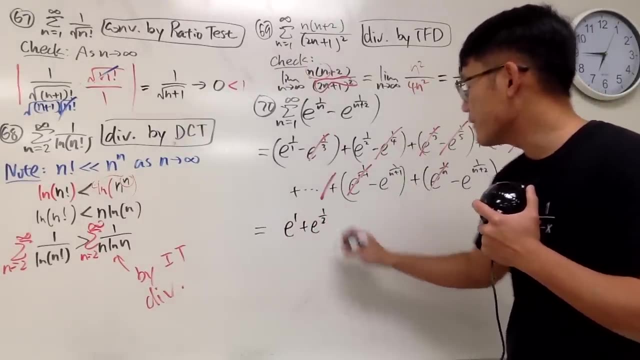 And so on, Right, And of course, it keeps on going forever. All right, Now this is the term that we have to look at, which is e to the first power plus e to the 1 half, And we have to look at minus, e to the 1 over m plus 1.. 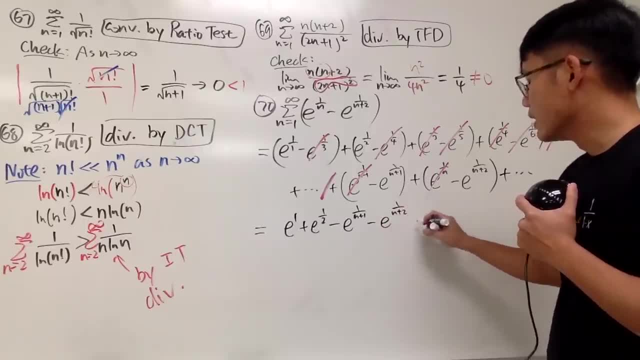 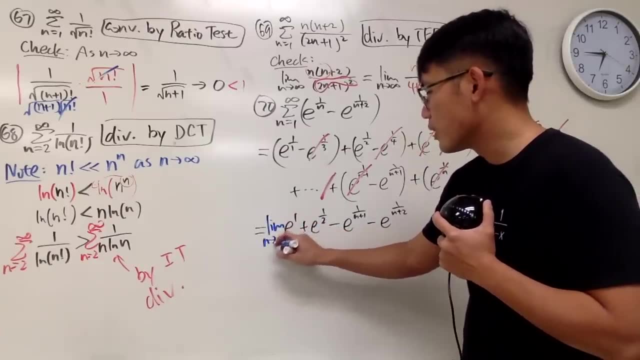 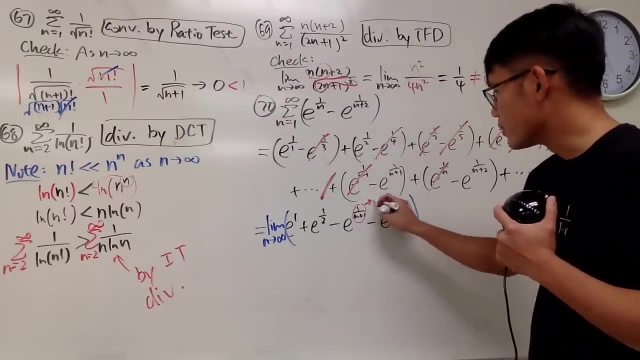 And then minus e to the 1 over m plus 2.. This is it. This is the nth partial sum formula, And then we are going to take the limit, As n goes to infinity, And the beauty of this is that the power goes to 0.. 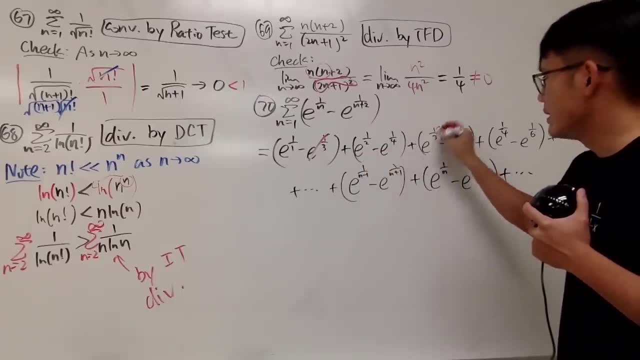 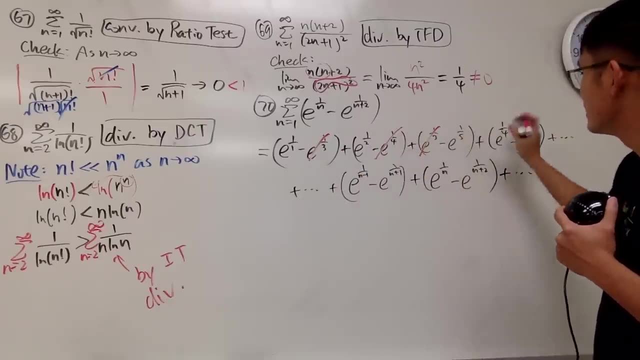 Not this, not this, But this Right. this is a jump. This right here stays, This right here, cancelled out With that. Okay, so notice: This right here will also be cancelled out With something after this right here, And this right here will be cancelled out With something after that. 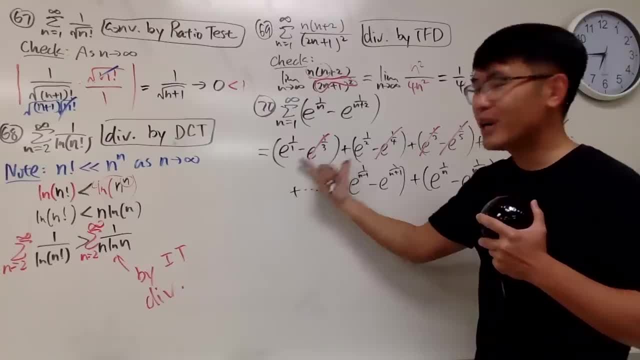 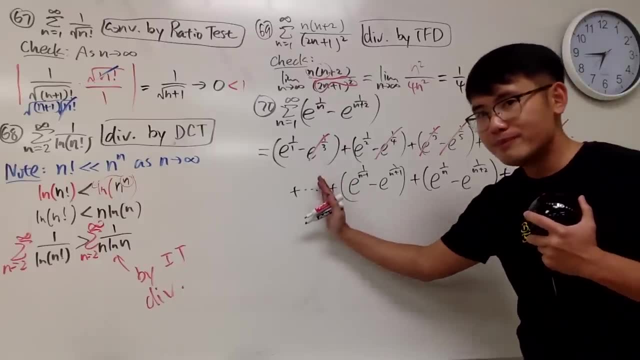 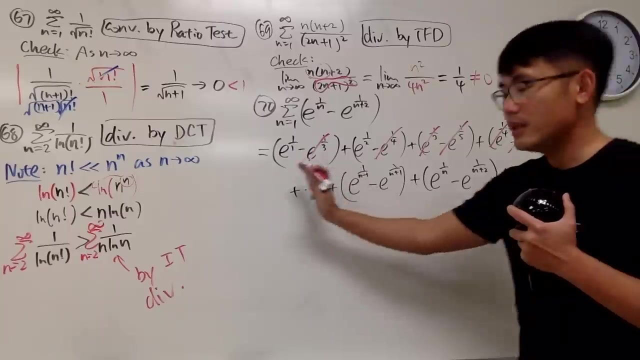 And the truth is you will have two terms Remained, Two terms remained, And you also have the following: Somewhere right here, Right, somewhere right here. Somewhere right here actually Will cancel out this guy first. Let me see, Yeah, somewhere in the front It's going to have some guy cancel out this. 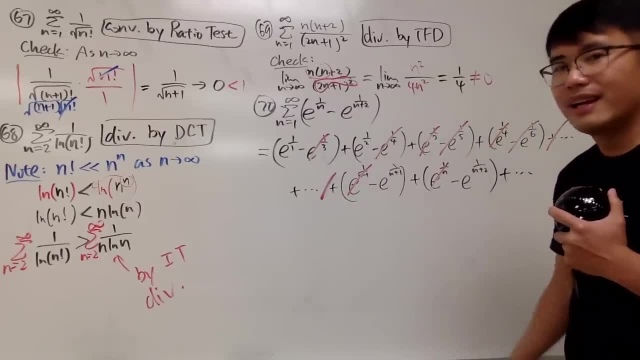 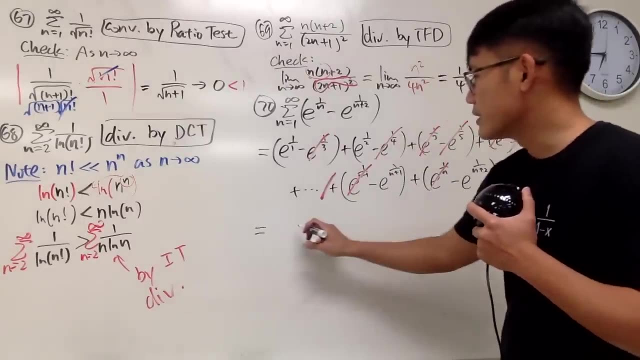 And then the term right before this: This guy is going to cancel out with this guy, And so on, And of course, it keeps on going forever. Now, this is the term that we have to look at, Which is e to the first power Plus e to the one half. 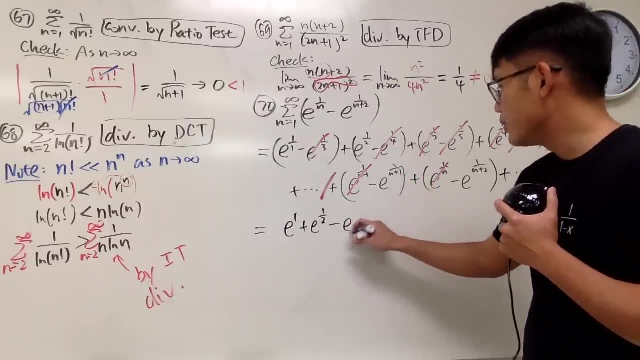 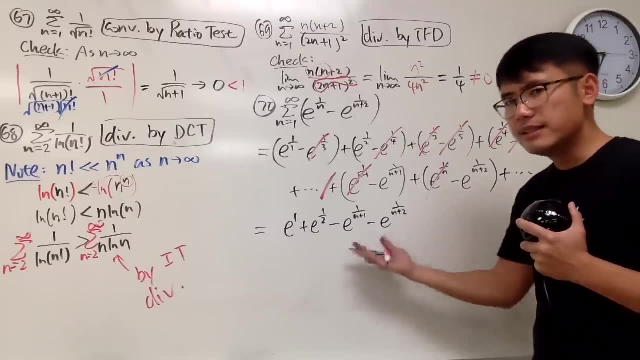 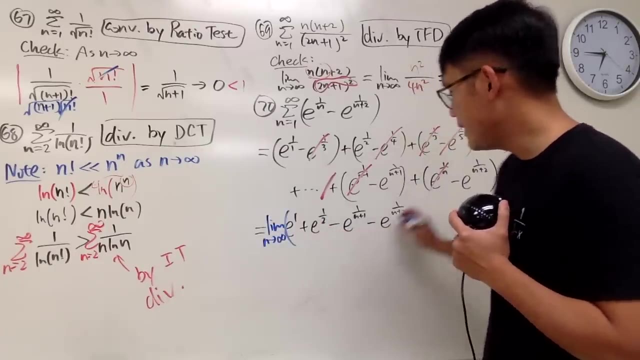 And we have to Look at minus e to the one over N plus one, And then minus e to the one over N plus two. This is it, This is the partial sum formula, And then we are going to take the limit As n goes to infinity, And then 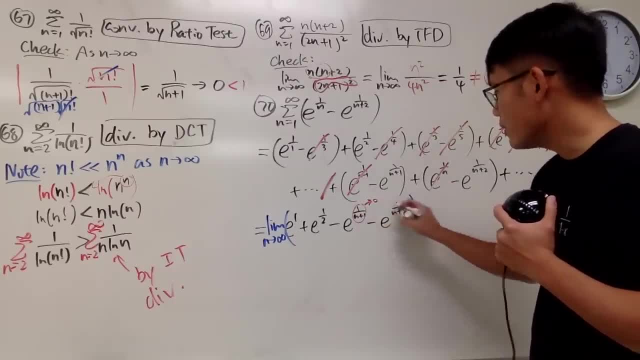 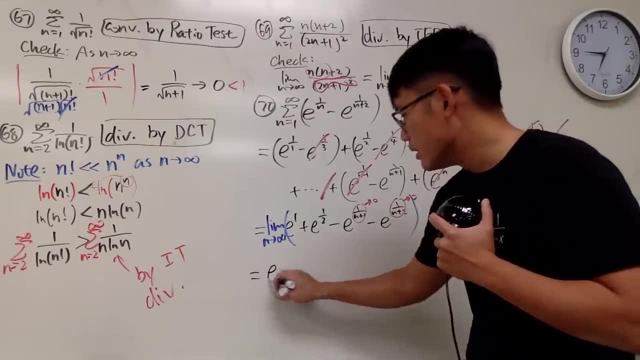 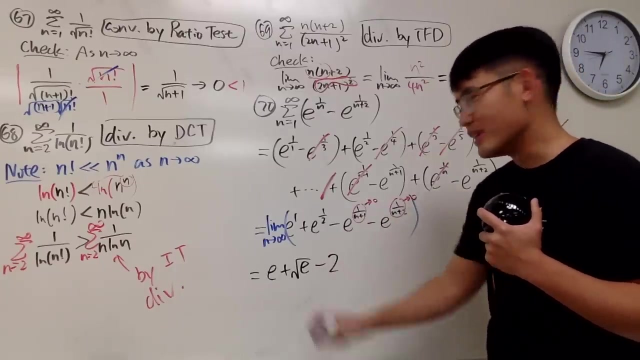 The probability of this is that The power goes to zero. The power goes to zero, So this is actually just one and one. So in the end, This is e, And if you want, you can write it down as square root of e, Just for fun. And then this is one one, so it's minus two. 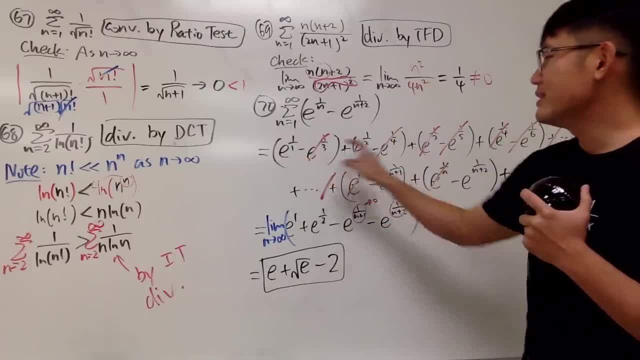 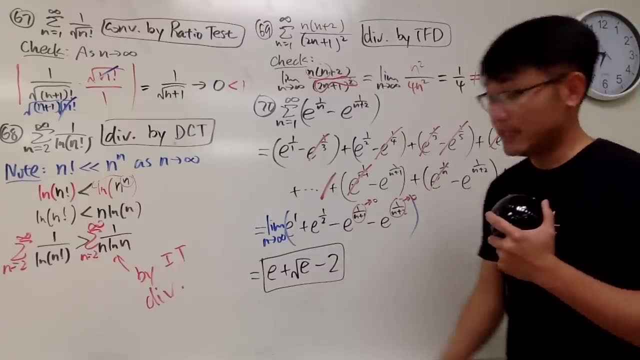 Minus one, minus one, so minus two. So this is it. Again, if it's off by two, This first two terms will survive And you will have two more terms that you have to subtract. So that's the idea: 30 more to go. Ok, now I'm counting down. 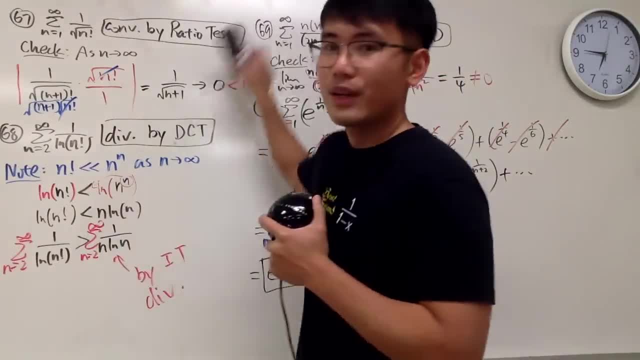 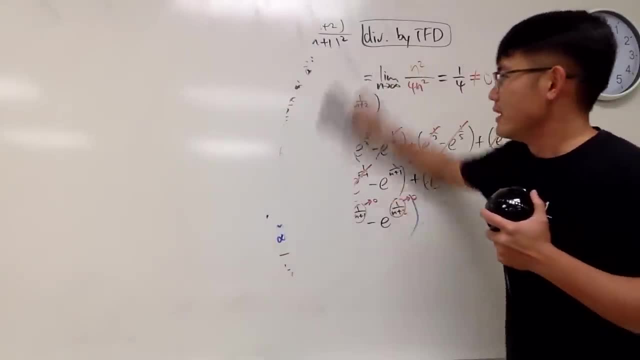 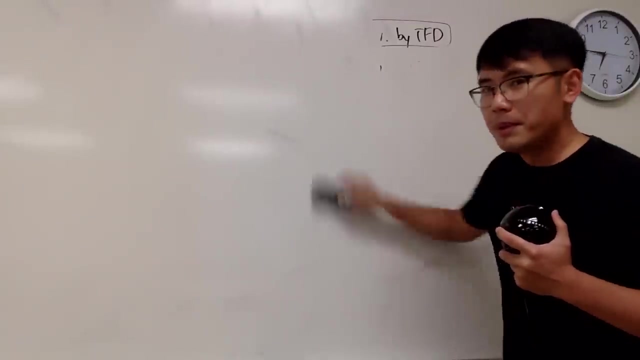 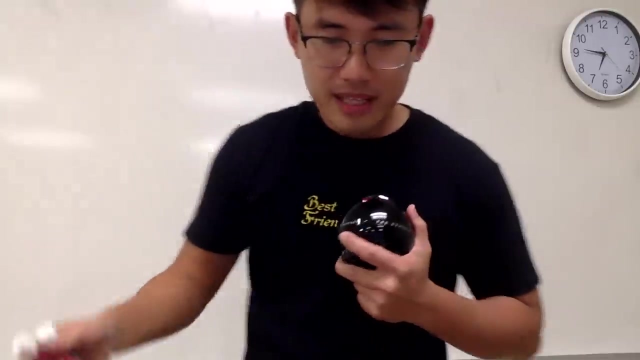 Ok, Ok, We can do this, We can do this, We can do this. If you guys Find this video helpful, Please let me know. The more people like this, The more I will do this, So give me a like so I know that you actually like it Right Now. number. 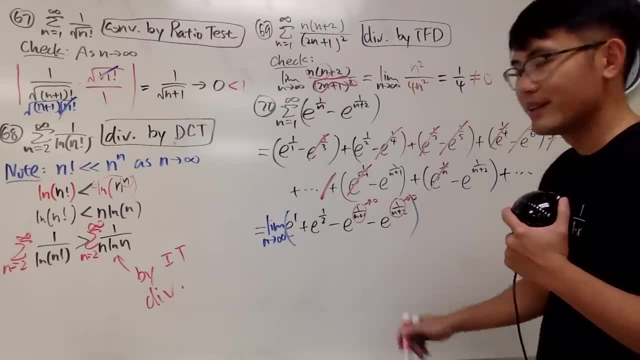 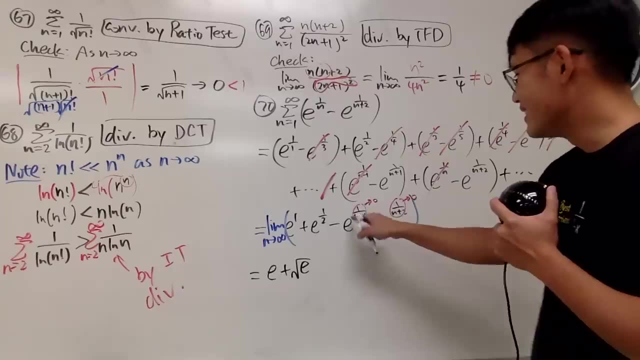 The power goes to 0.. So this is actually just 1 and 1.. So in the end, this is e And, if you want, you can write it down as square root of e, just for fun. And then this is 1, 1.. 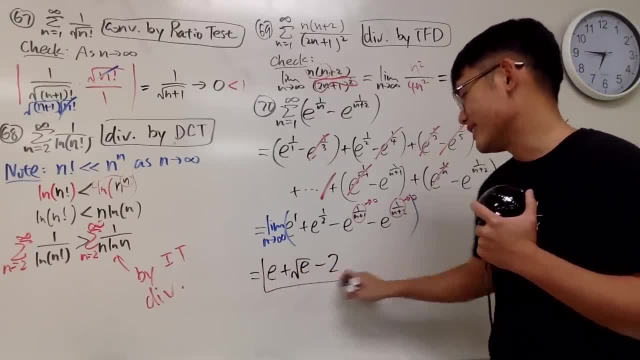 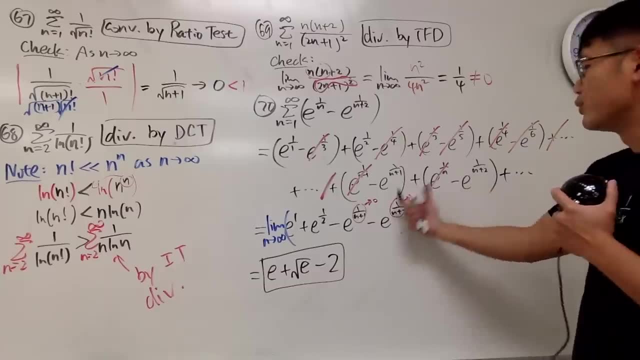 So it's minus 2.. Minus 1,, minus 1,, so minus 2.. So this is it. Again, if it's off by 2, these first two terms will survive And you will have two more terms that you have to subtract. 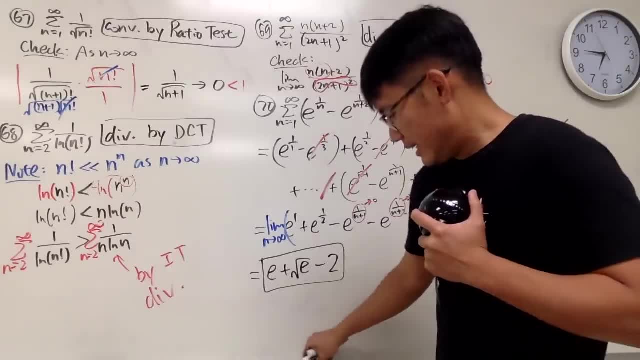 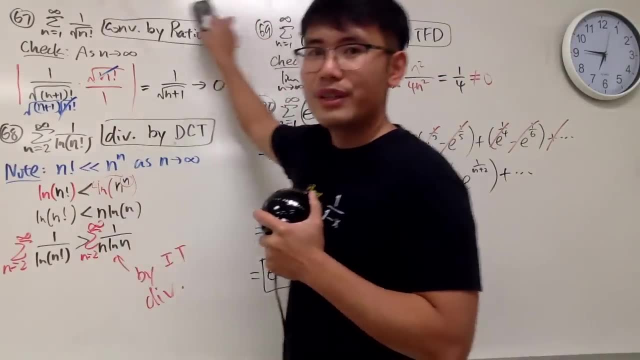 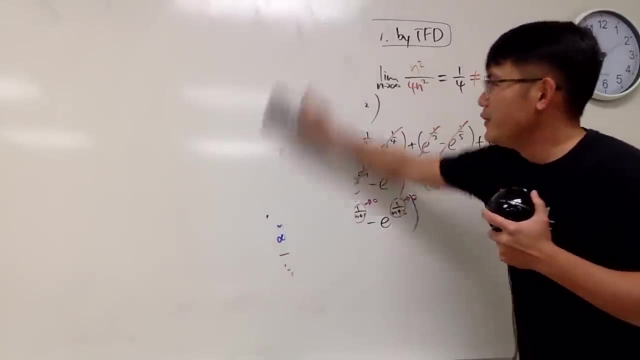 So that's the idea. So that was number 70.. 30 more to go. Okay, now I'm counting down. Okay, okay, okay, We can do this, We can do this, We can do this. If you guys find this video helpful, please let me know. 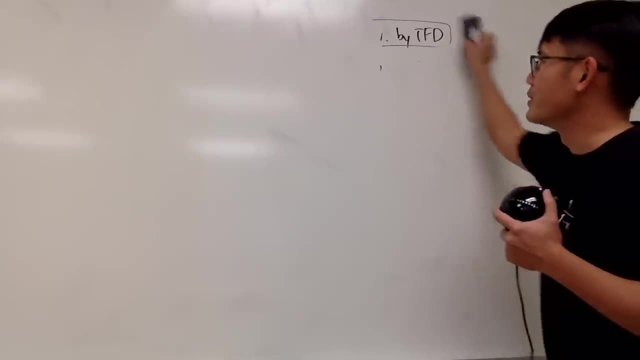 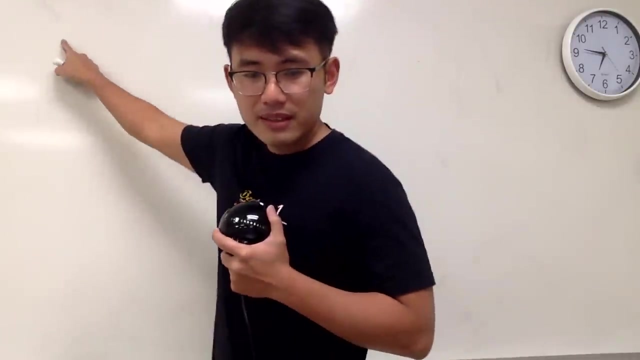 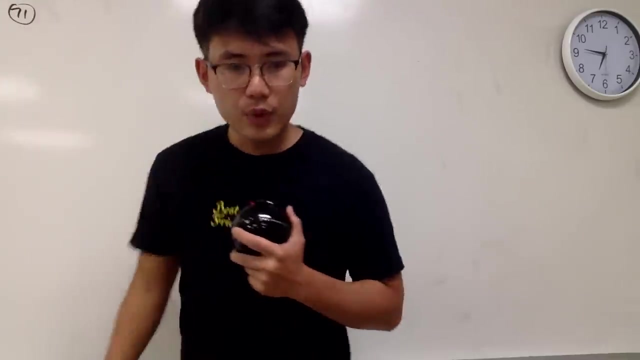 All right, The more people like this, the more I will do this. So give me a like, So I know that you actually like it. All right Now, number 71.. Right here. All right, here we go. We are going to find the sum as n goes from 3 to infinity. 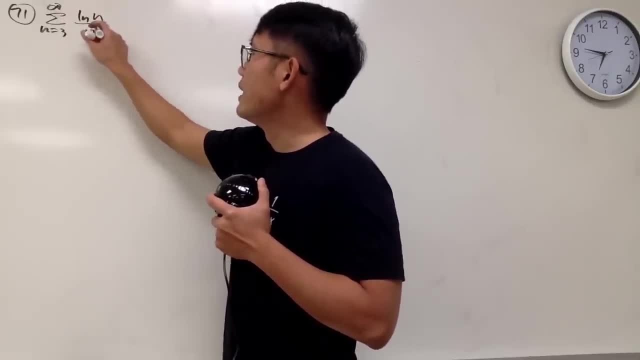 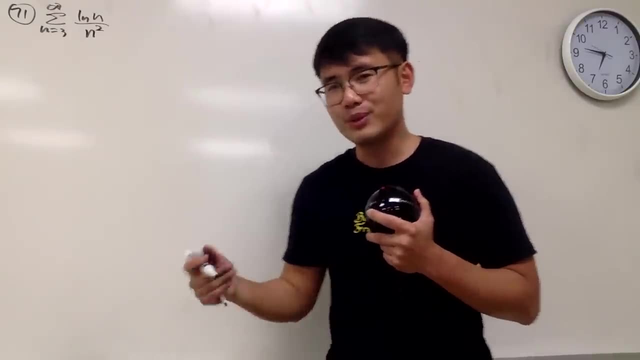 Now to find the sum, just like the series, to see if this converges or not. n to the second power, like this: If you would like, you can do some integration by parts. You can do the integral test. I will leave that to you. 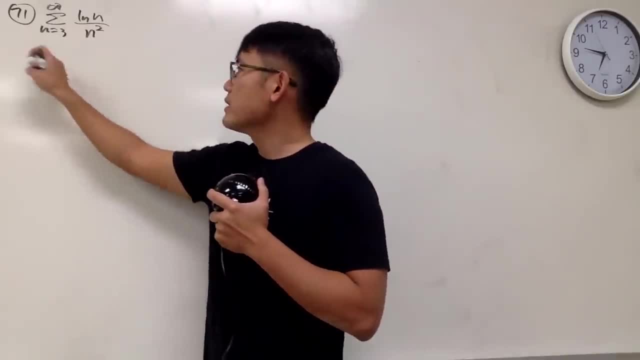 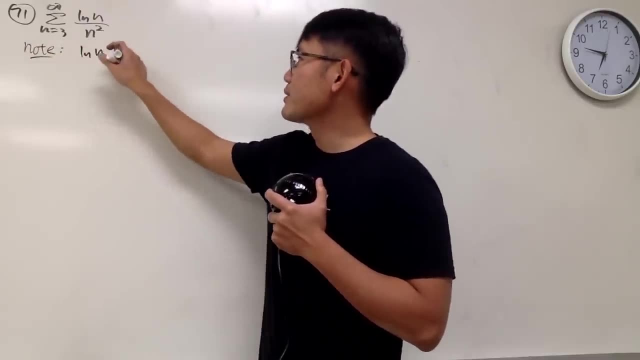 But I will do this. So here is the deal. First of all, note again, here is the deal. okay, ln n is actually less than well, this is true, but I want to use square root of n right here. 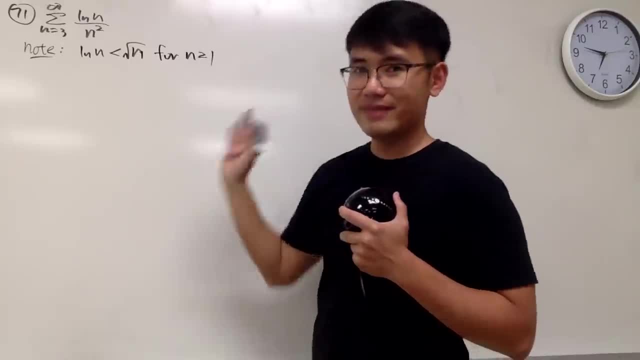 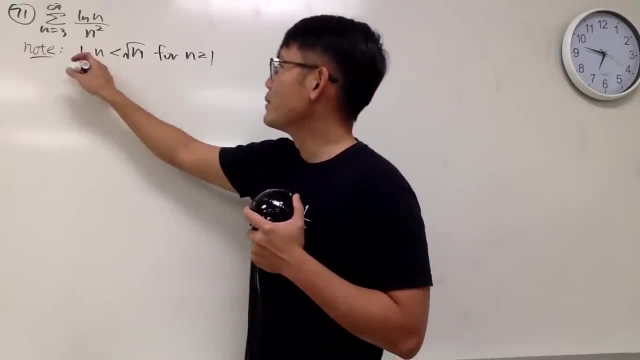 And this is true for n greater than or equal to 1.. So that's great. So you could have started with 1, if you would like. Now we just have to do a few more things. Check this out. I will just have to divide both sides by n squared. 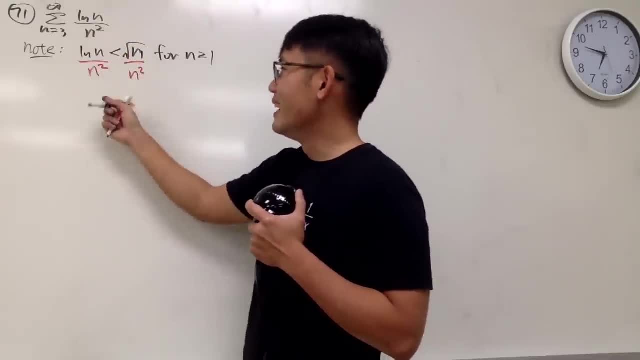 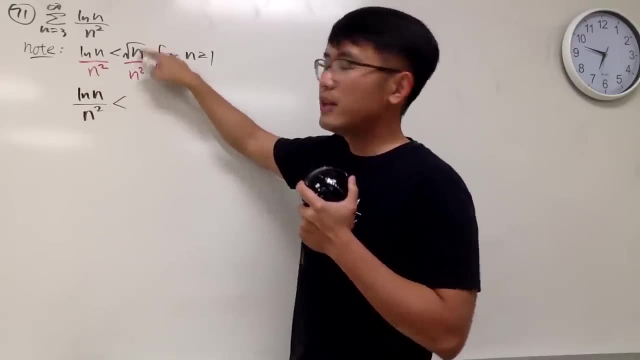 Why? Because that's what we want. So notice: on the left-hand side we have ln, n over n squared, And on the right-hand side, this is n to the one-half power, This is n to the second power. Work this out. 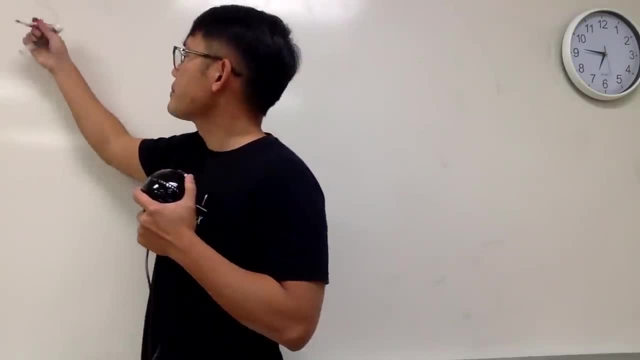 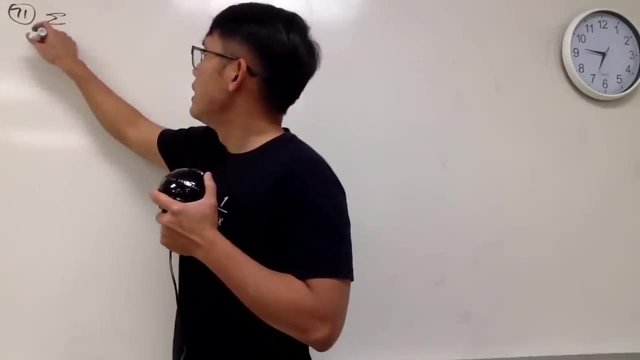 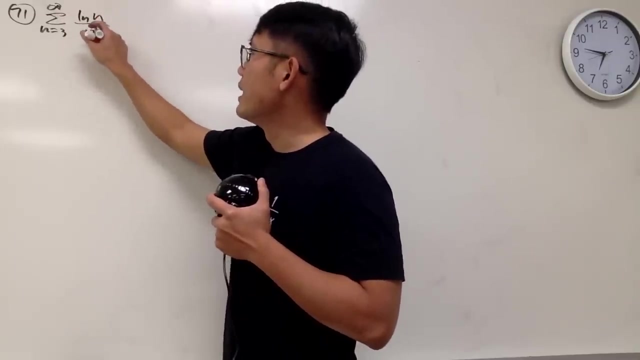 71. Right here. Alright, here we go. We are going to find the sum As n goes from three to infinity, As n goes from three to infinity. Now find the sum, just like the series, To see if this converges or not. n to the second power, like this: 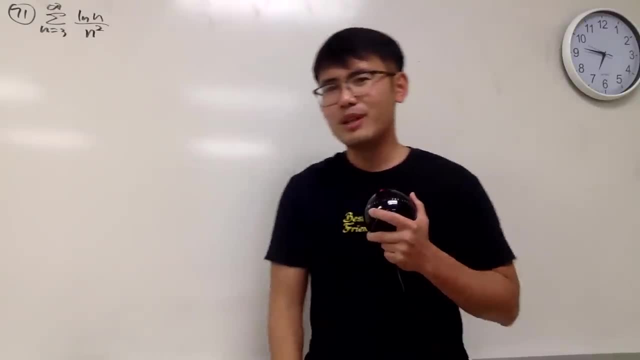 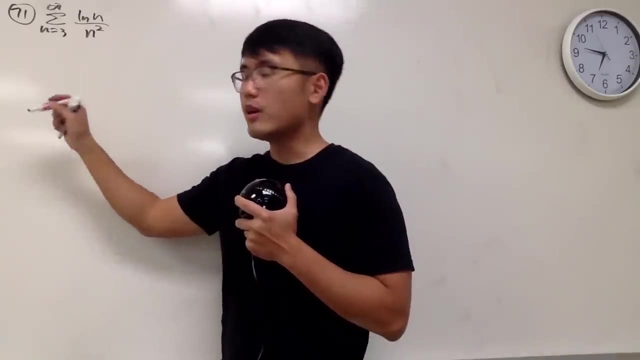 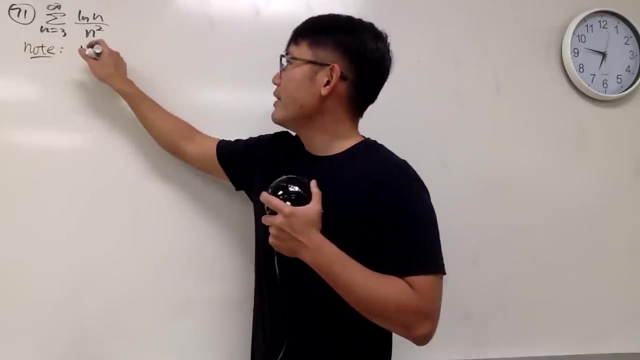 If you would like, You can do some integration by parts And do the integral test. I will leave that to you, But I will do this. Here is the deal, First of all. Note again, Here is the deal: ln. n is actually less than Well, this is true, But I want to use square root of n. 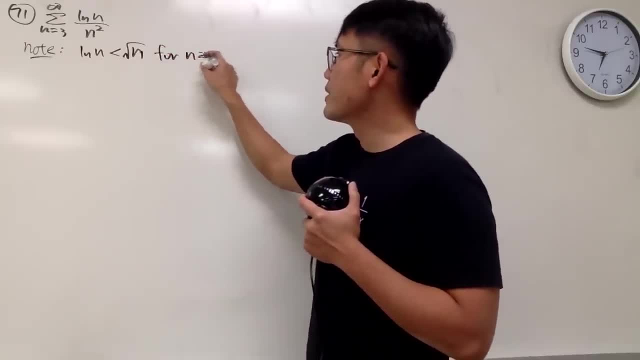 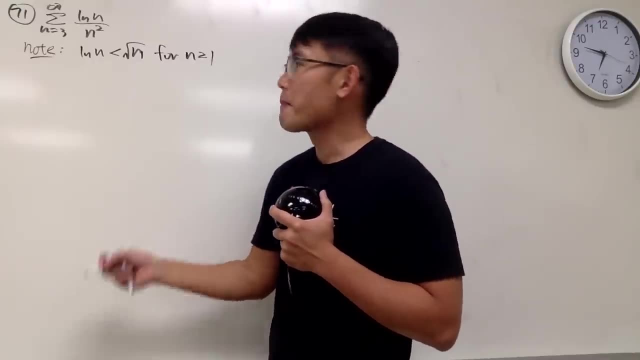 Right here, And this is true for n greater than or equal to one. So that's great. So you could have one if you would like. Now we just have to do a few more things. Check this out. I will just have to divide both sides by n squared. 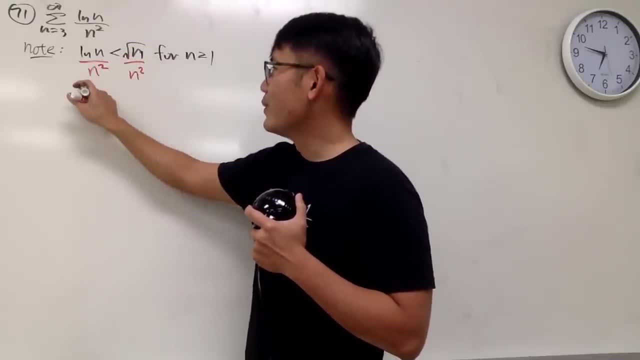 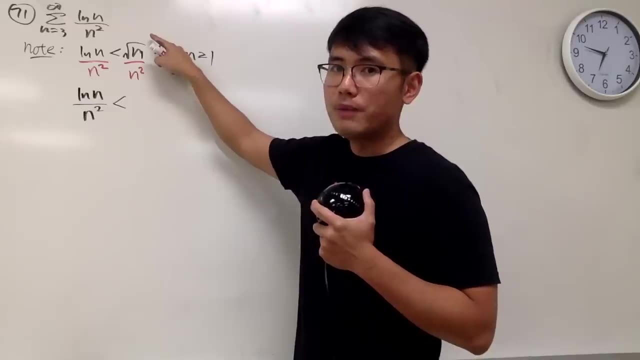 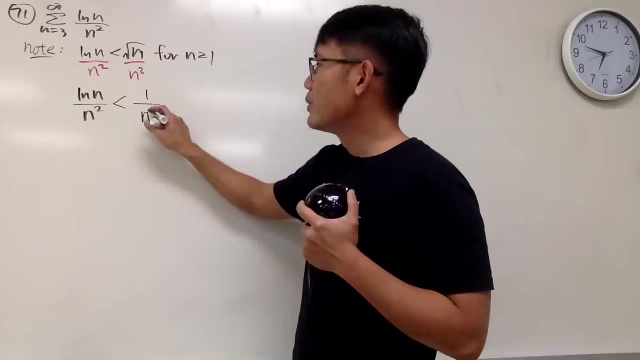 That's what we want. So notice: on the left hand side We have ln, n over n, squared, And on the right hand side, This is n to the one half power, This is n to the half, This is n to the second power. Work this out, You end up with one over. 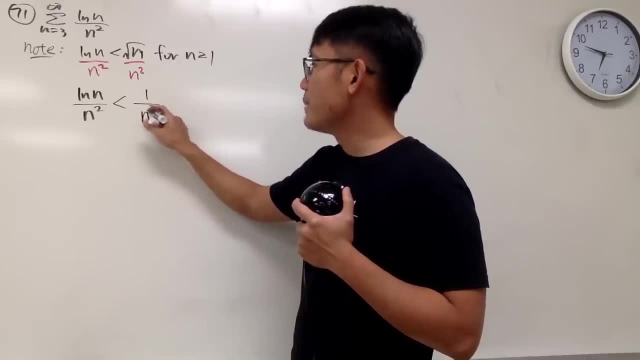 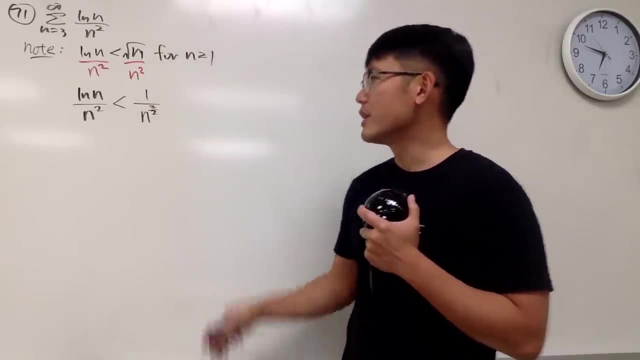 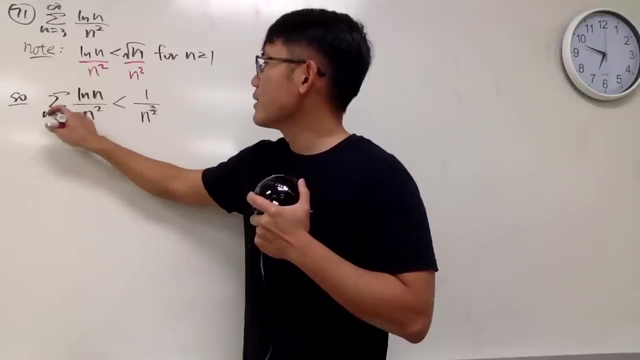 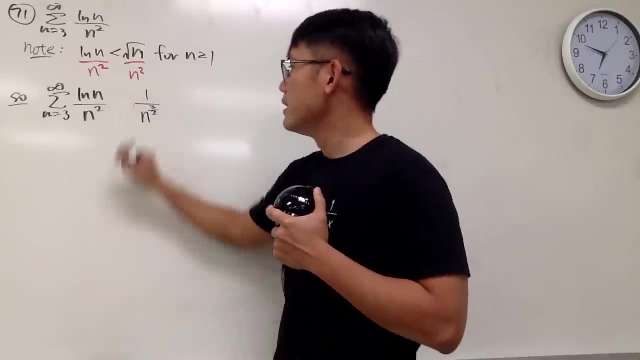 n to the Three half power. Right, One minus two, I mean one half minus two, You get negative three half. And now, of course, So We get the sum as n goes from Three to infinity. And of course, let's put this down On both sides Like this: And: 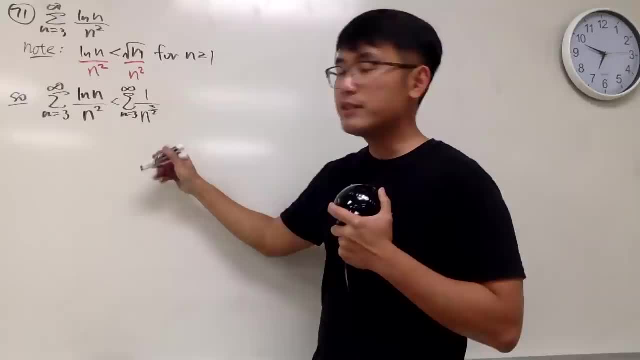 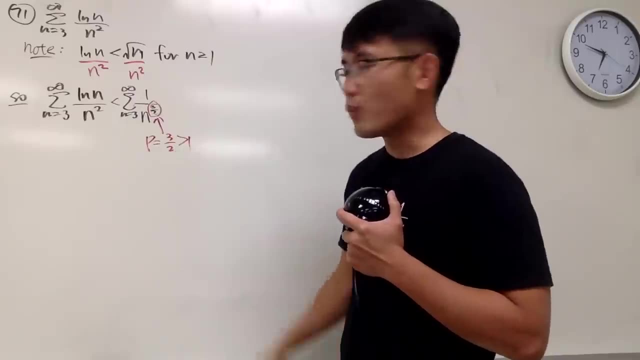 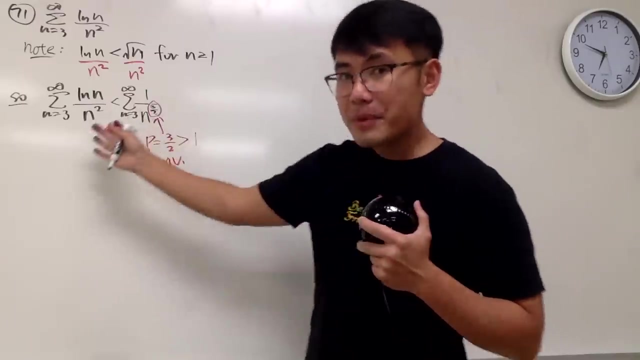 n is equal to three, to infinity. This right here. Take a look, Don't we have a p series- Yes, we do- Which is greater than one. So does it converge or not? It converges. So let's put that down And I'll come here And we will say this right here: 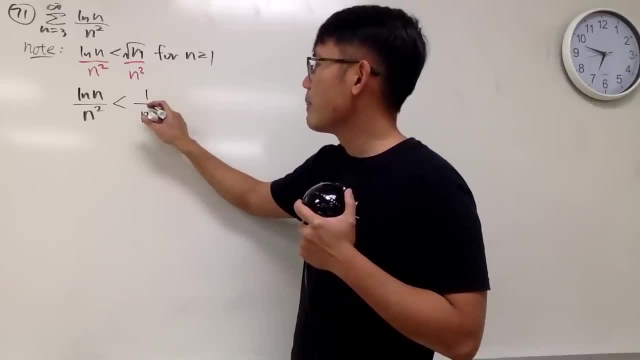 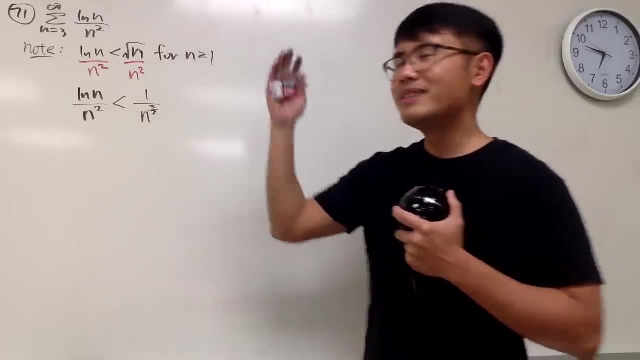 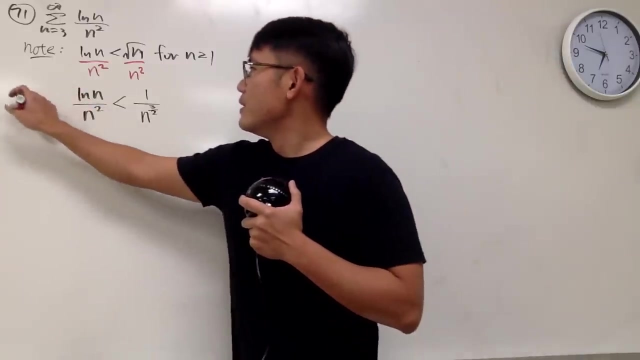 You end up with 1 over n to the three-half power, Right, Yeah, 1 minus 2.. I mean 1 half minus 2.. You get negative 3 half and you have this. And now, of course, so we get the sum as n goes from 3 to infinity. 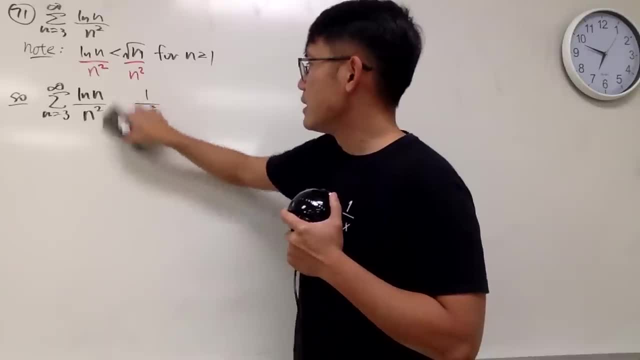 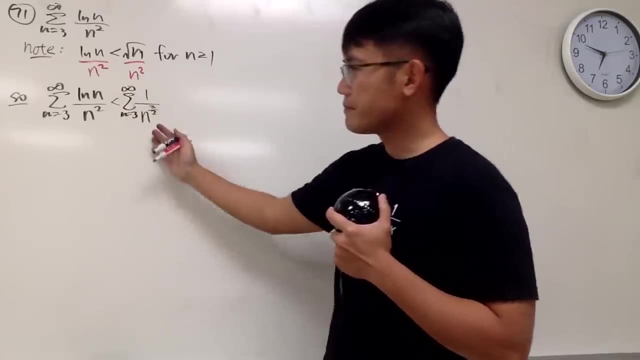 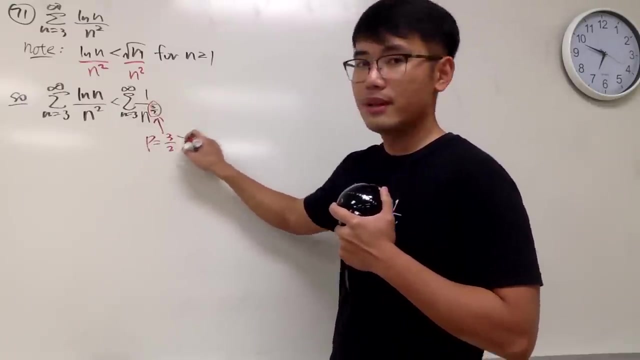 And, of course, let's put this down on both sides like this: And n is equal to 3, to infinity. This right here. take a look, Don't we have a p-series? Yes, we do. It's 3, half, which is greater than 1.. 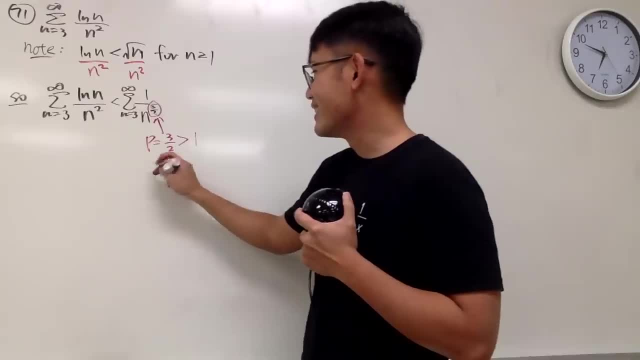 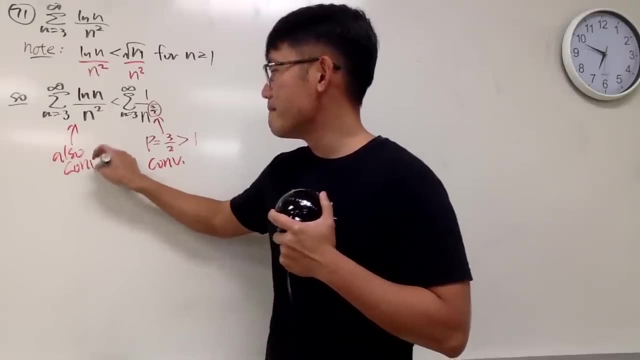 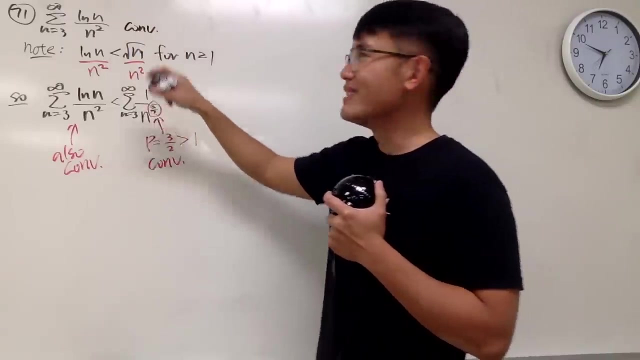 So does it converge or not? This right here converges, So let's put that down And I'll come here and we will say: this right here also converges. Come back here and just say: this right here converges as well by the direct comparison test. 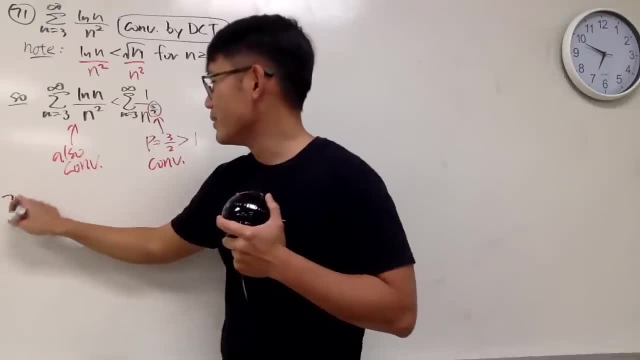 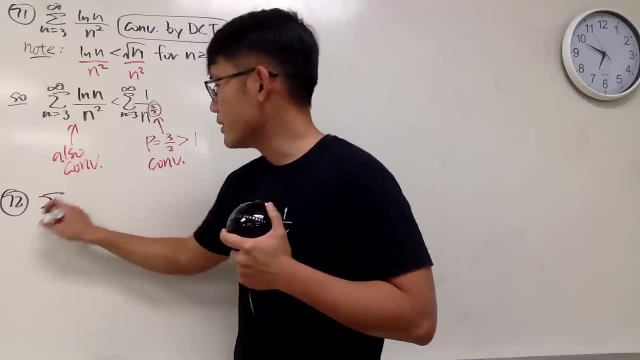 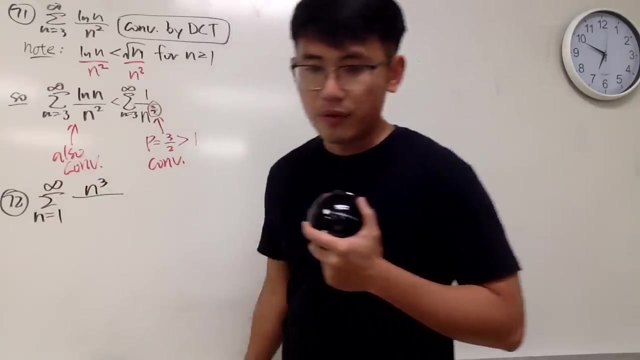 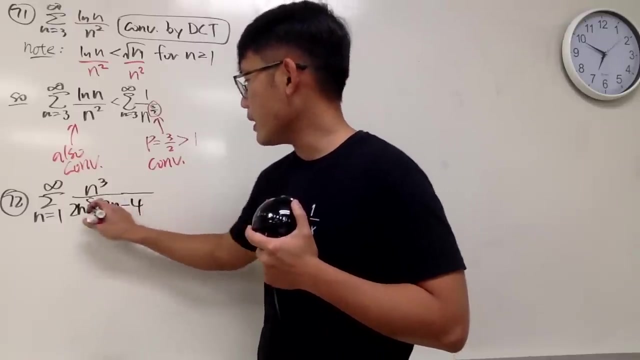 And with that we are done. So nice, huh 72.. So this is the sum, as n goes from 1 to infinity, n to the third power over 2, n to the fifth power plus 3, n minus 4, like this: 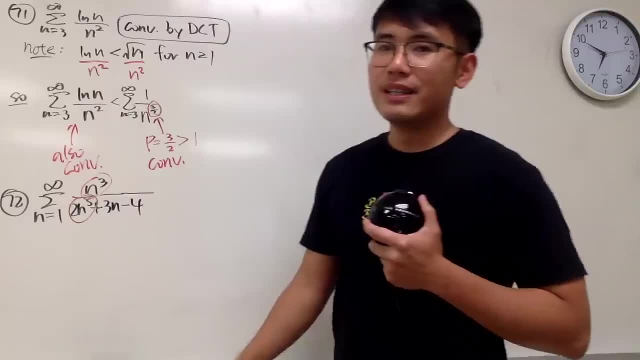 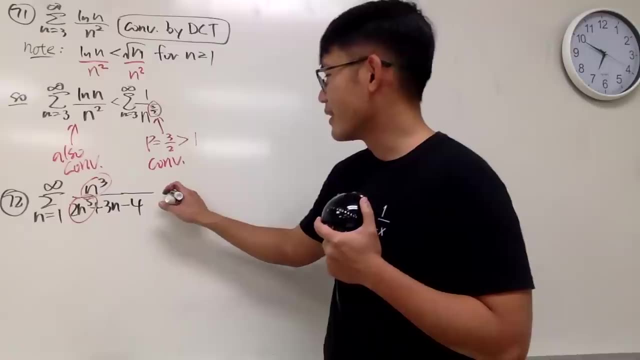 Well, you can see the deal. Pick this, pick that And you end up with, say, 1 over n, squared Right. So just work this out. Let me tell you This right here: converges by some kind of comparison test. 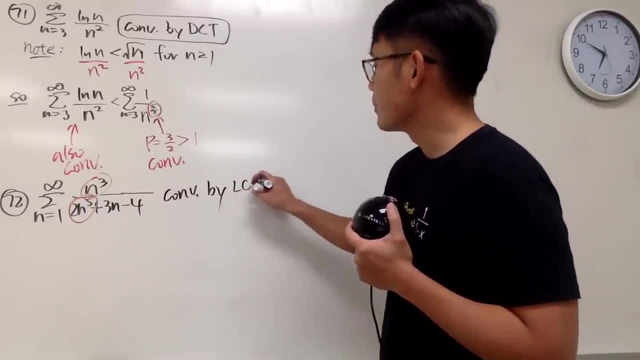 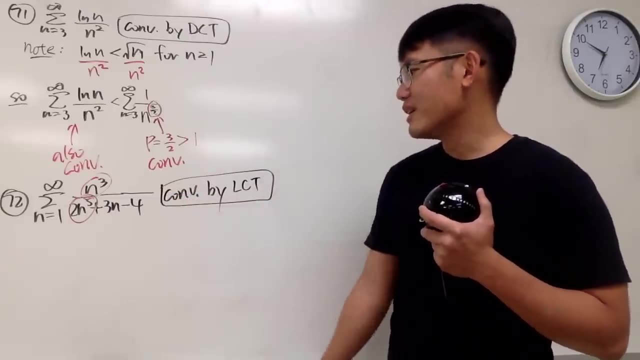 And of course it might be easier if you just use the limit comparison test for this, Because if you want to work out the inequality, sometimes it may not work out so well, But I think limit comparison test works out pretty well. But of course if it works out then it's up to you as well. 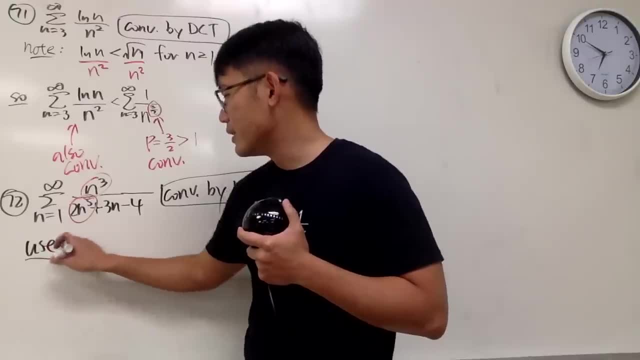 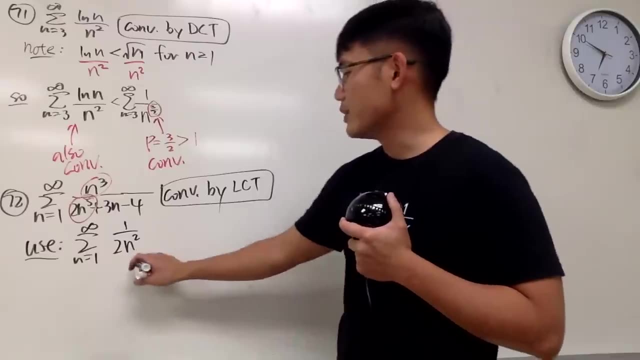 So I'll just tell you: use the sum as n goes from 1 to infinity. This over that which is just 1 over 2, n squared like that which is convergent. So this right here, p is 2, which is greater than 1.. 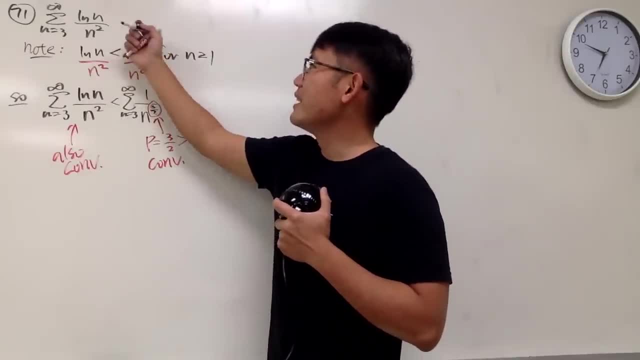 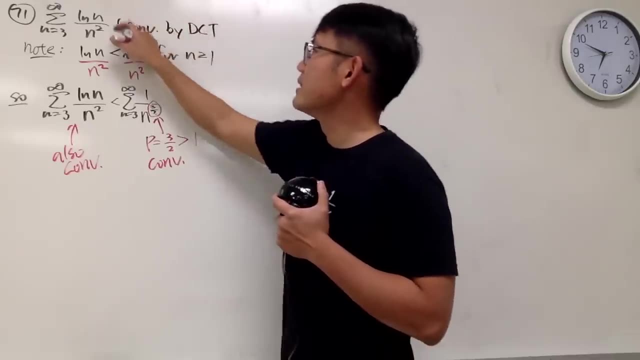 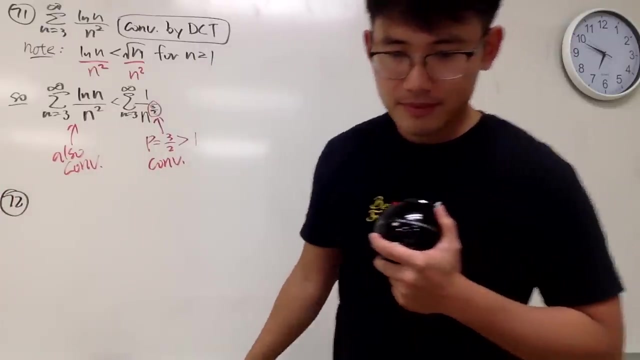 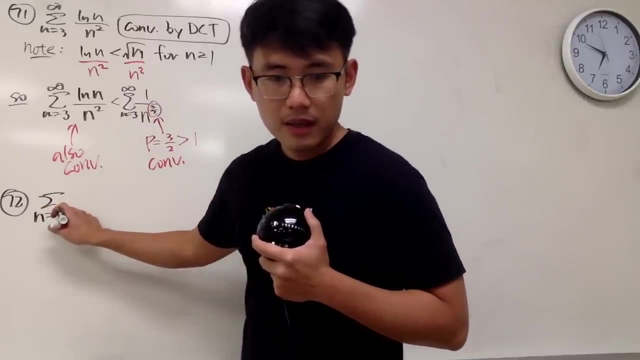 Also converges. Come back here And just say this right here: Converges as well By the direct comparison test, And with that We are done. So nice, huh, Now 72. So this is the sum. So this is the sum As n goes from One to infinity. 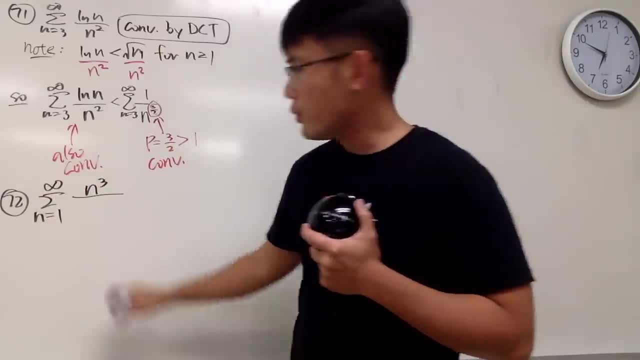 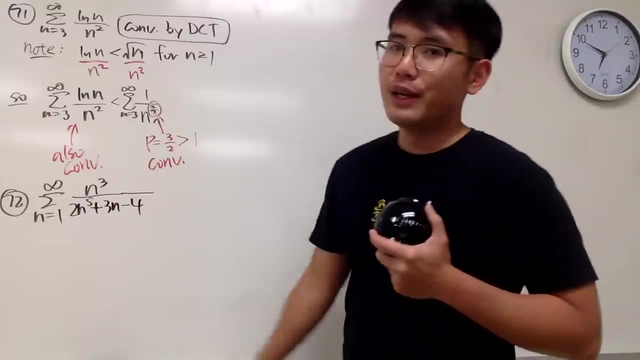 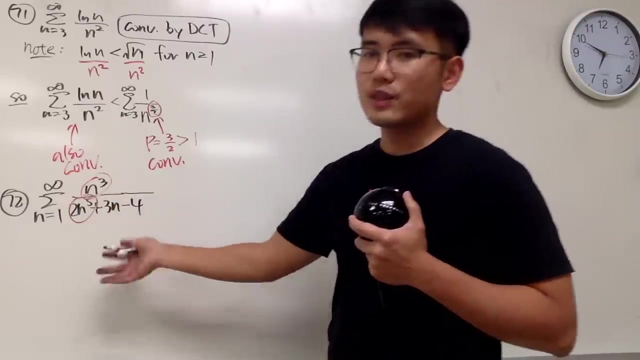 n to the third, power Over two. n to the fifth power Plus three n Minus four, Like this. Well, you can see the deal. Pick this, pick that And you end up with like One over n squared part, right. So just work this out. Let me tell you this right here: converges. 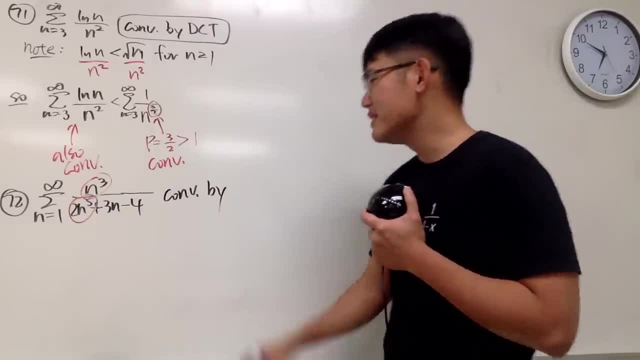 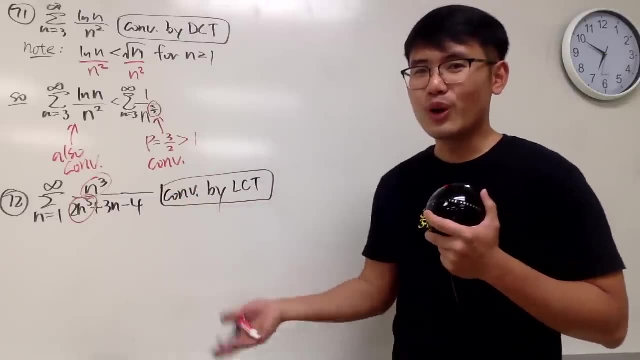 By some kind of comparison test. And of course it might be easier If you just use the limit comparison test For this, Because if you want to work out the inequality, Sometimes it may not work out so well. But I think limit comparison test works out pretty well, But of course if it works out. 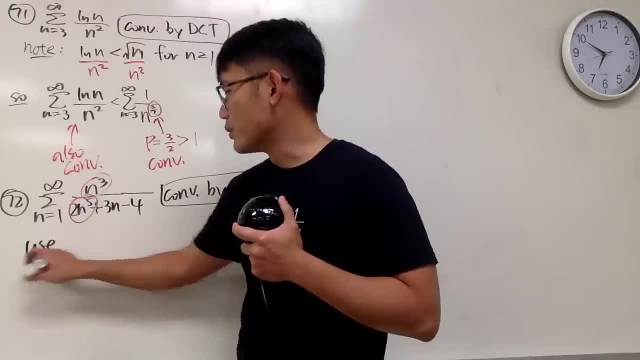 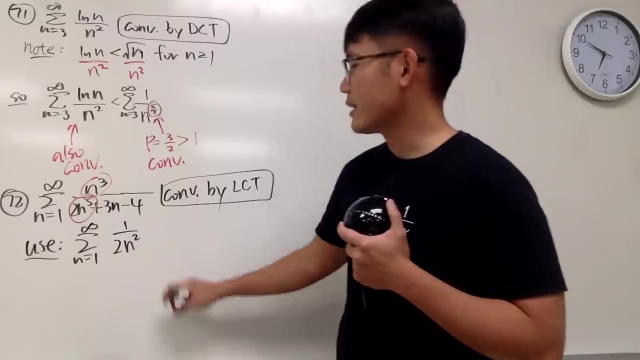 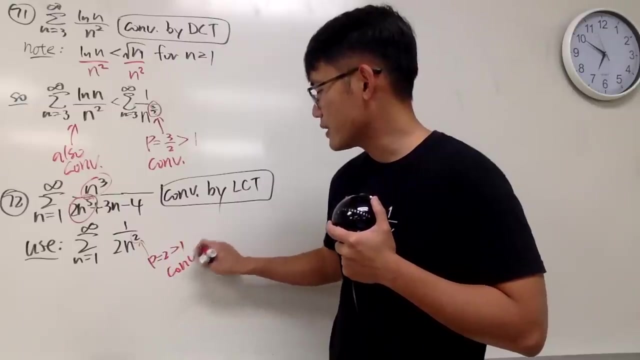 It's up to you as well. So I'll just tell you: Use the sum As n goes from one to infinity, This over that, which is just one over two. n squared Like that, which is Convergent: Here p is two which is greater than one, It converges. 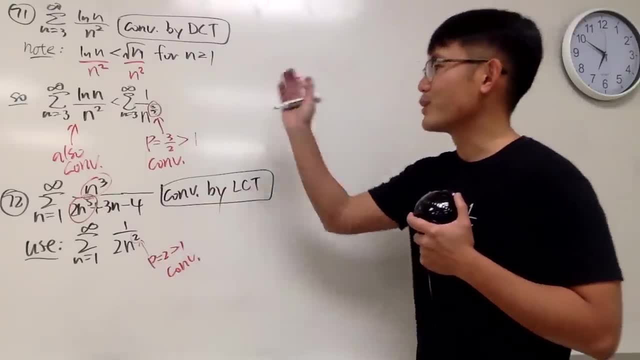 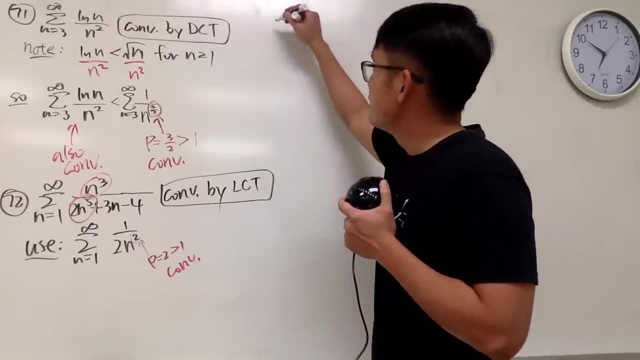 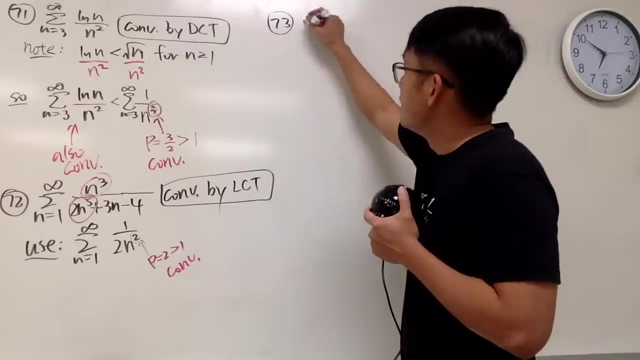 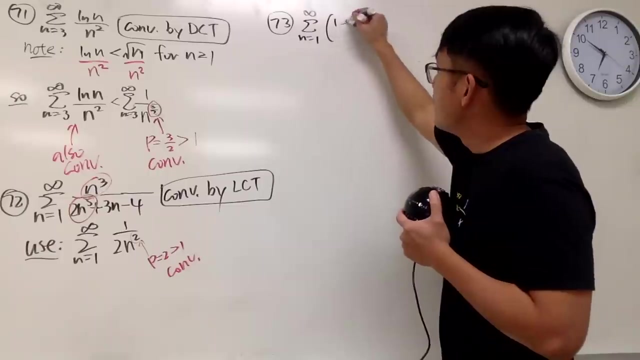 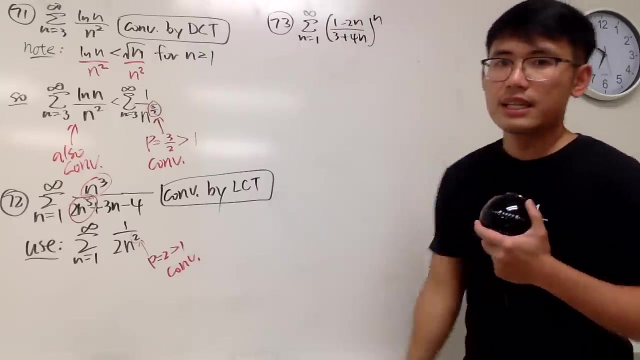 Right, so use this And compute the inequality So you'll be able to work that out. Okay, Seventy Three, Alright, Sum as n goes from one to infinity And we have a Big expression, One minus two, n, Three plus four, n Raised to the nth power, Like this: 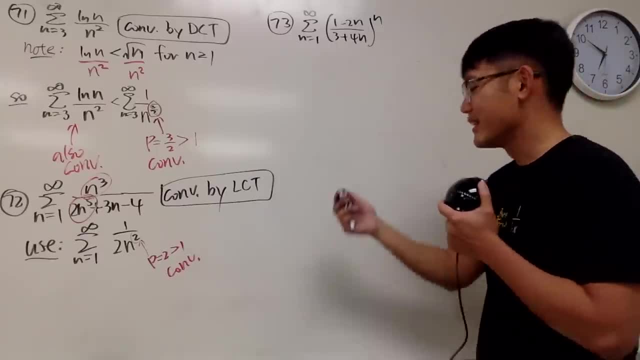 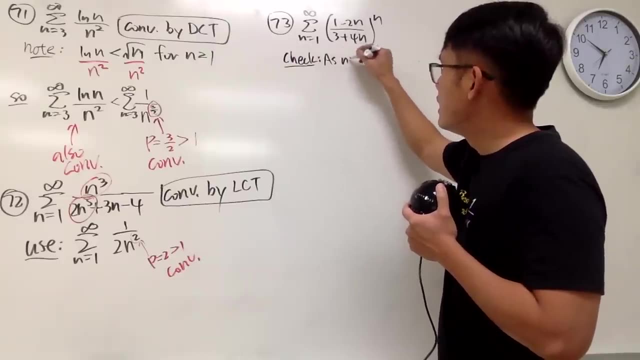 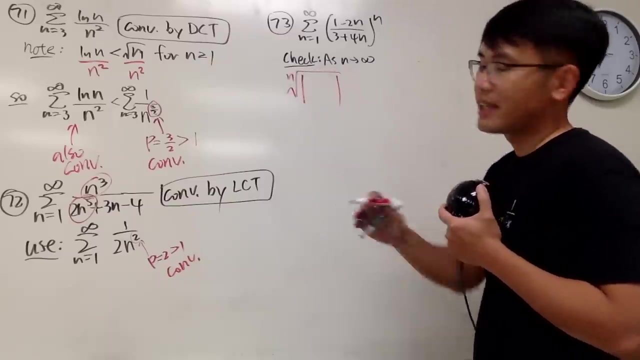 Now n in the power Root test, Very nice. So go ahead and check, As n goes to infinity, And I will just Take the nth root and then Absolute value. In this case we may need to have the absolute value, But we'll see. You see, this is one minus. 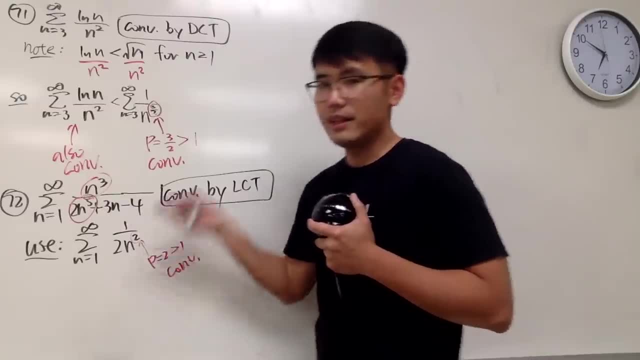 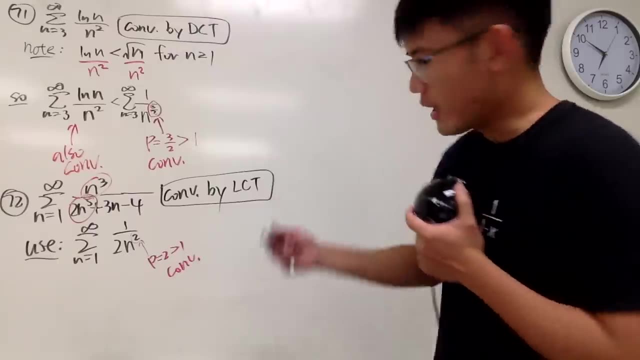 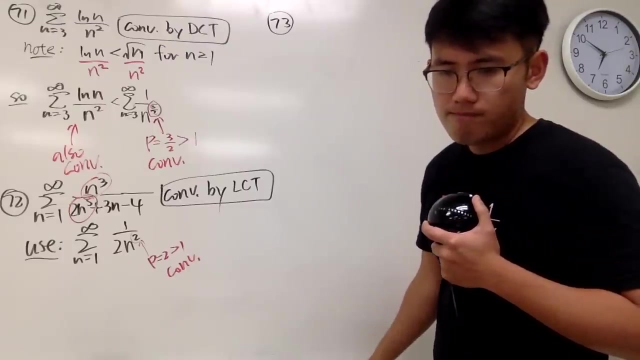 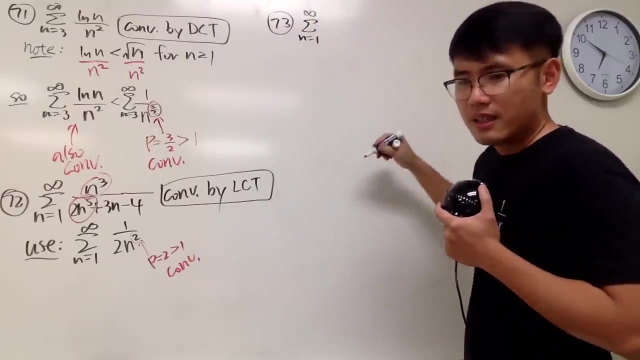 It converges Right. So use this and compute the inequality and all that, So you will be able to work that out. OK, 73.. All right, Sum as n goes. As n goes from 1 to infinity, And we have a big expression. 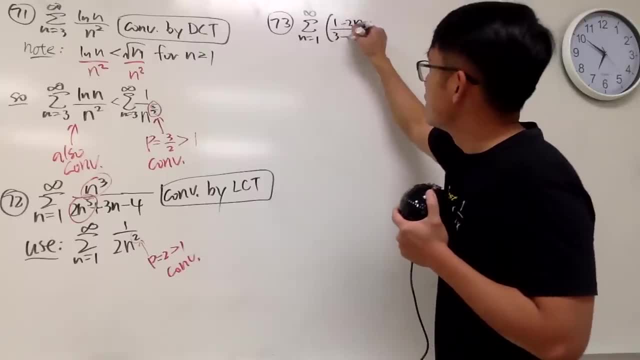 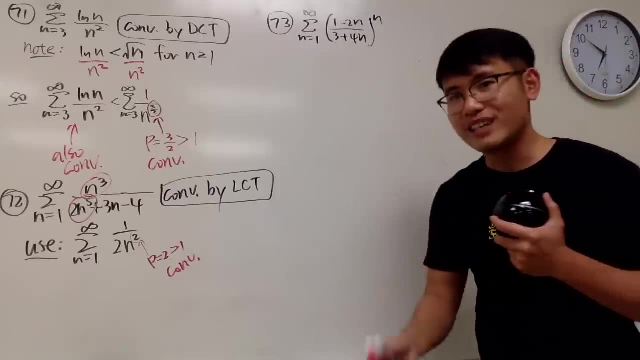 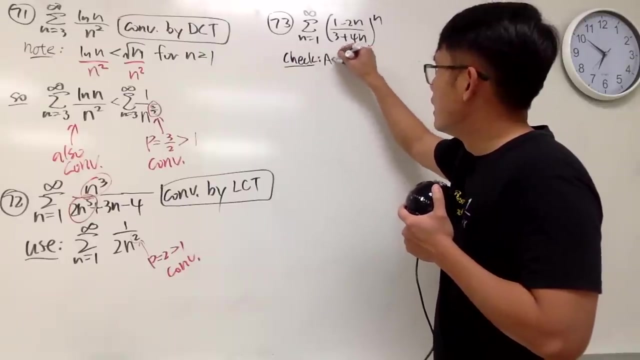 1 minus 2n over 3 plus 4n, raised to the nth power like this: Now n in the power root test. Very nice, huh. So go ahead and check as n goes to infinity And I will just take the nth root. 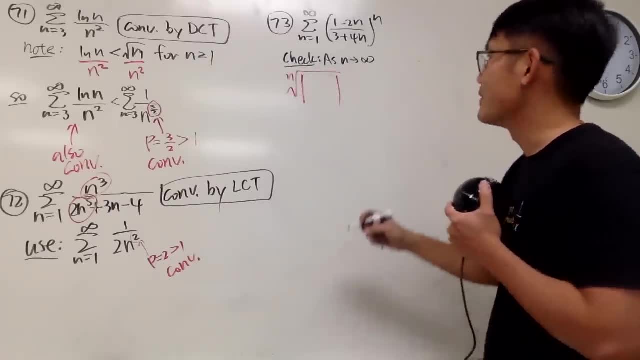 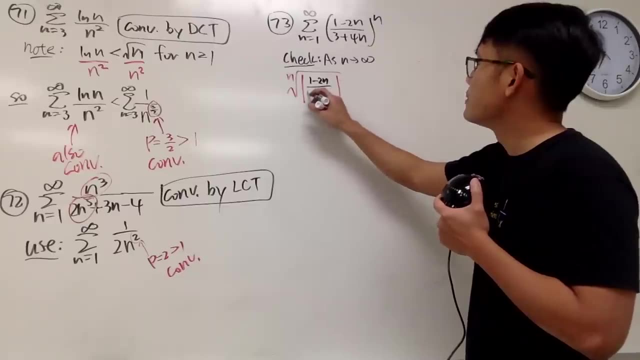 And absolute value. In this case, we may need to have the absolute value, But we'll see. You see, this is 1 minus 2n over 3 plus 4n, like this, And then we will just put this down to the nth power, like that. 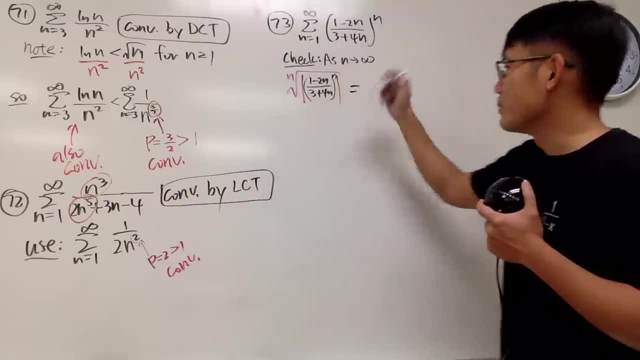 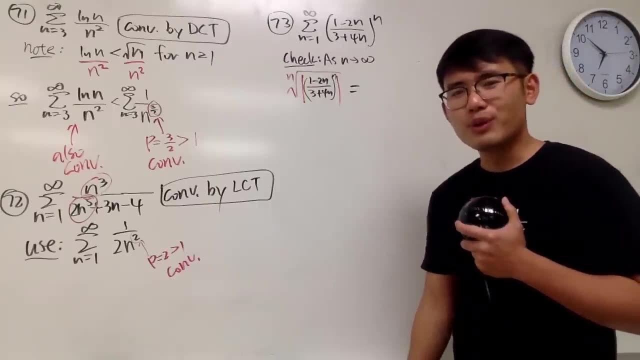 Well, of course, this n and i pretty much cancel out, So we get hm This right here. We actually get negative, though, So I think the absolute value does matter. huh, This is how we can take care of it. 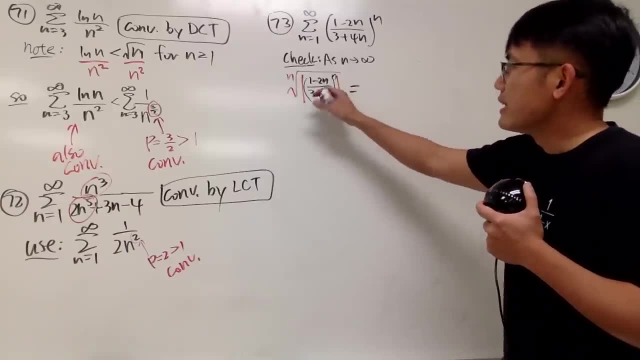 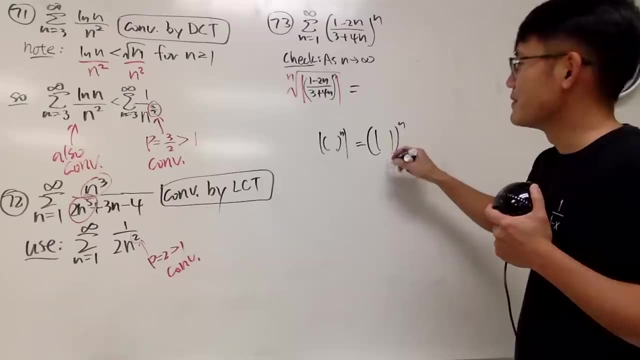 So, first of all, first of all, the idea is that the absolute value of some power, this is actually the same as the power outside of the absolute value. So this and that can be cancelled. No big deal, Right? No big deal. 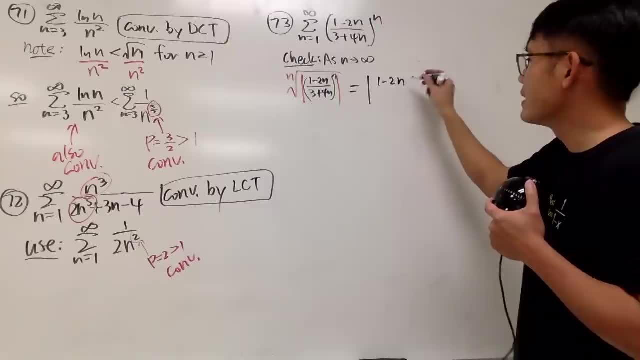 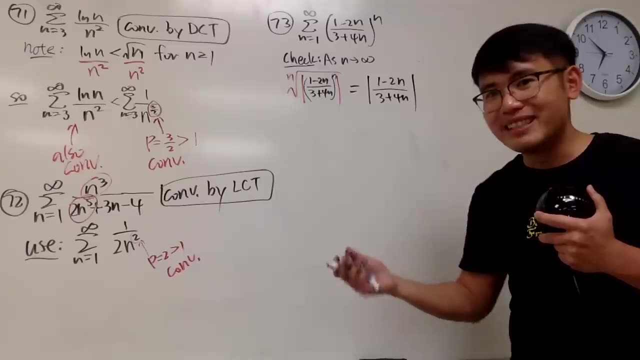 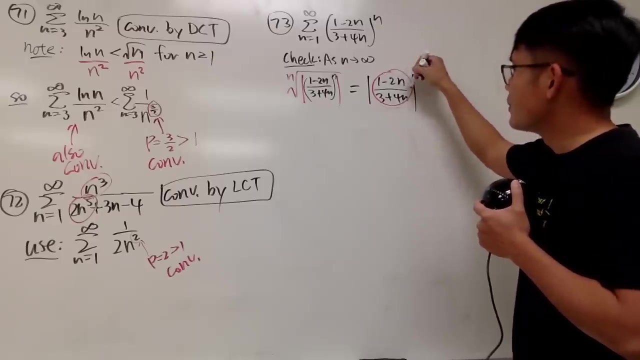 And I will still maintain the absolute value, which is 1 minus 2n over 3 plus 4n, like this. And now we just have to take the limit inside, And the limit inside is not that bad at all, because this is just going to be negative: 2n over 4.. 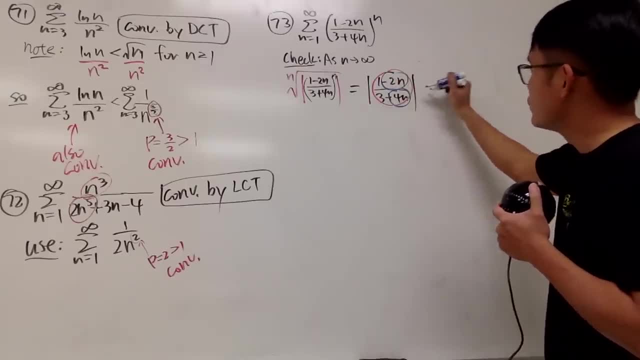 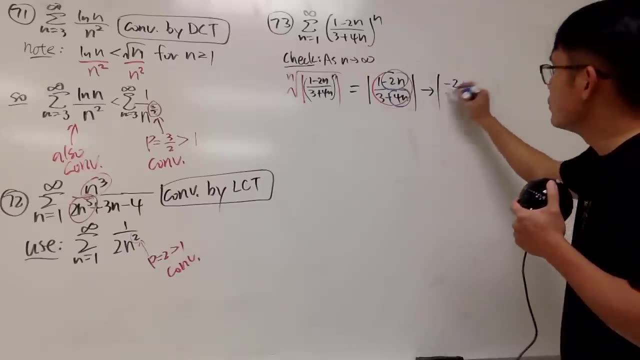 Take the limit inside and just consider this part and that part which we'll end up with. I'll just put down this right here: with the absolute value, We get negative 2 over 4n and n like this, And in the end you just do this inside out. 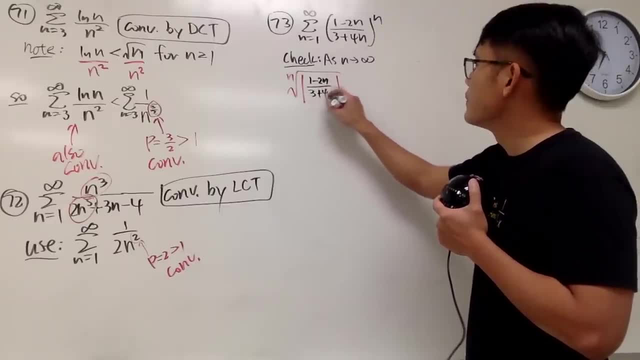 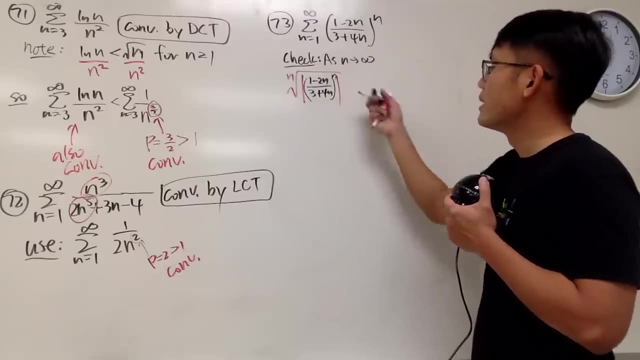 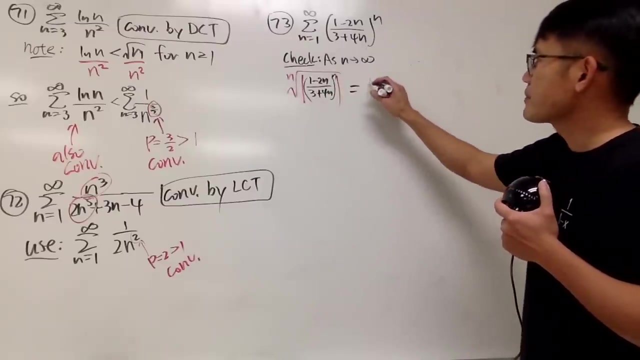 Two n over Three plus four n, Like this, And then we will just Put this down To the nth power, like that. Well, of course, the n and This n, and i pretty much cancel out. So we get This right here. We actually get negative, though, So I think the absolute value does matter. 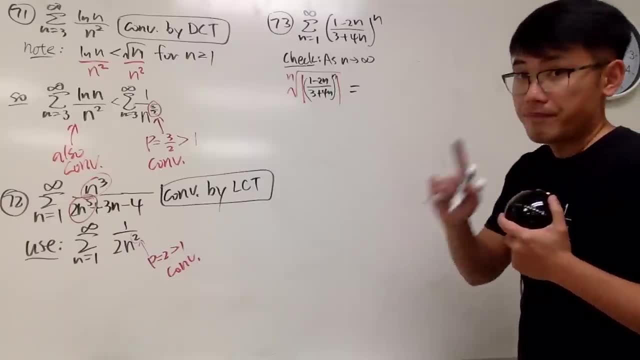 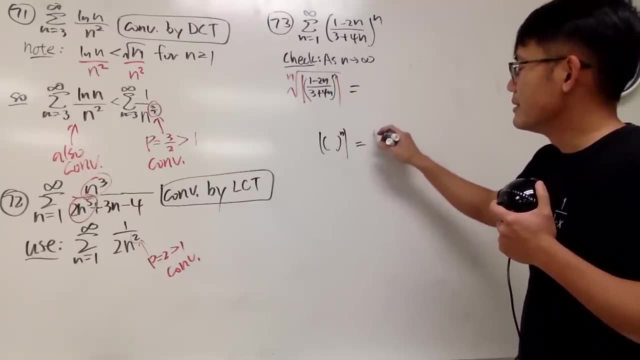 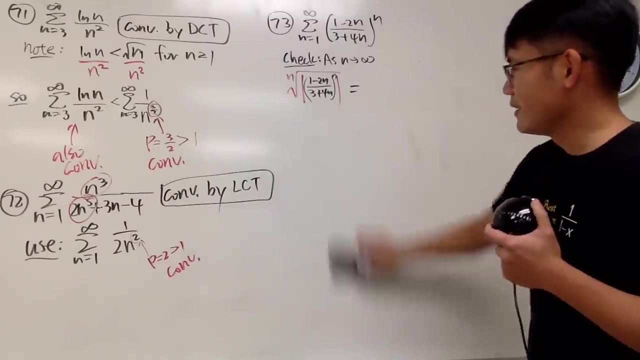 This is how we can take care of it. So, first of all, First of all, the idea is that The absolute value of some power, This is actually the same as The power Outside of the absolute value. So this and that can be cancelled, No big deal, And I will still maintain the absolute value. 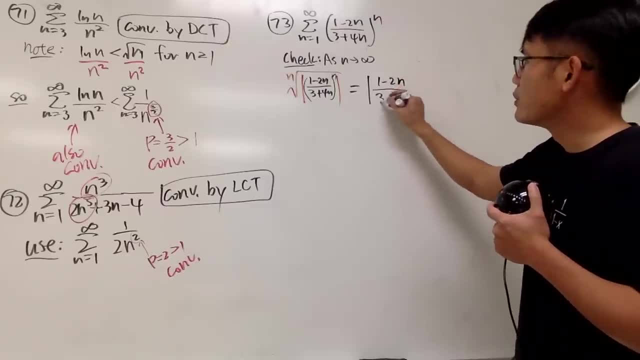 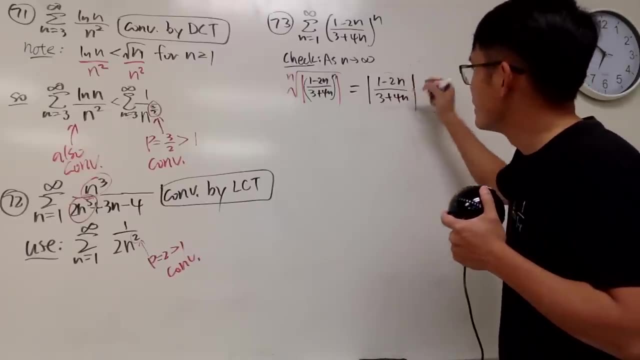 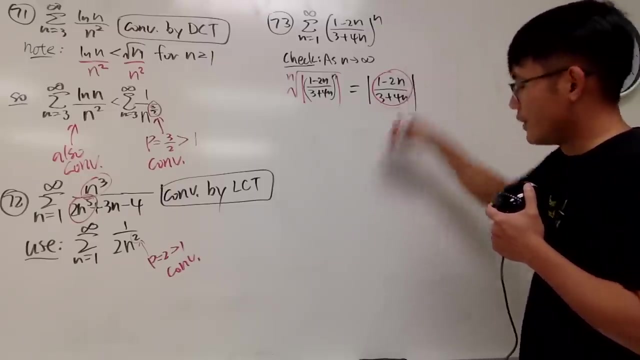 Which is one minus Two n over Three plus four n Like this. And now we just have to take the limit Inside, And the limit inside is not that bad at all, Because this is just going to be Two n over four. Take the limit inside And just consider this part and that part. 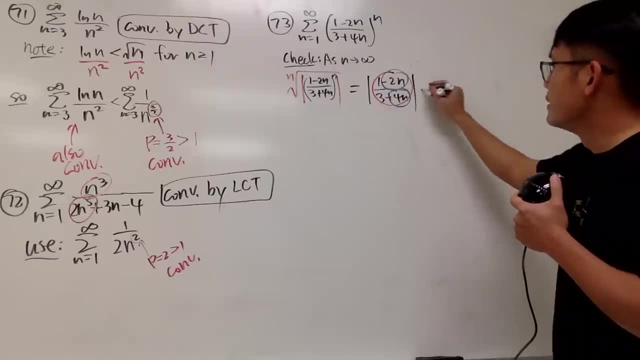 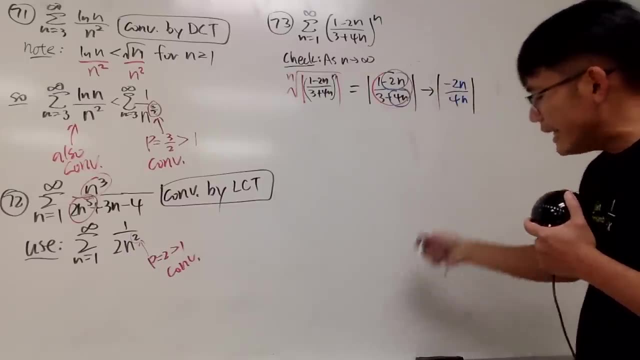 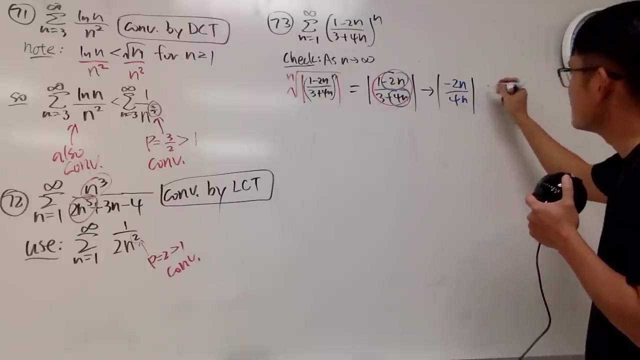 Which we will end up with. I will just put down This right here: With the absolute value, We get negative two over four, N and n like this, And in the end You just do this inside out. The absolute value is a continuous function, So you can just pretty much do that. 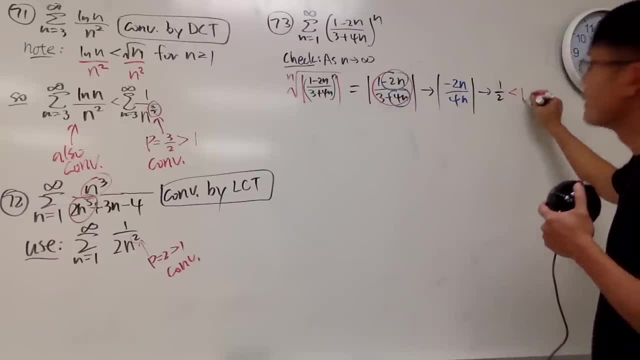 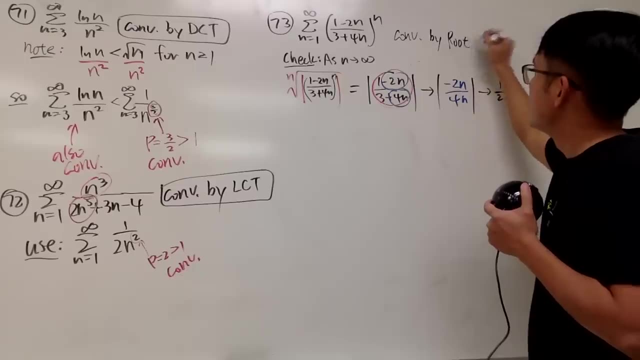 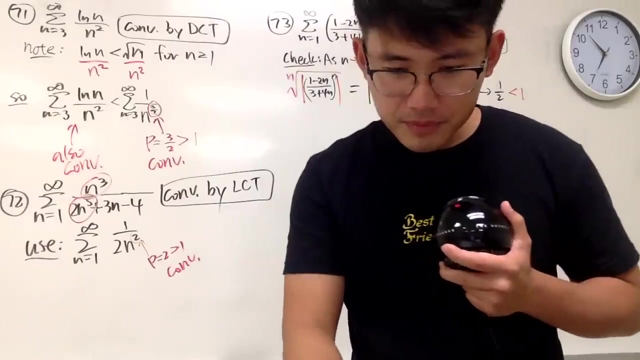 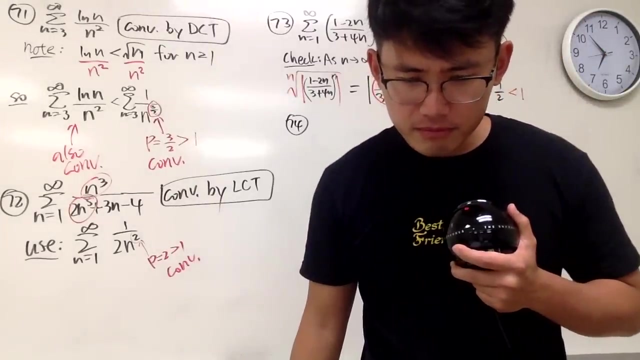 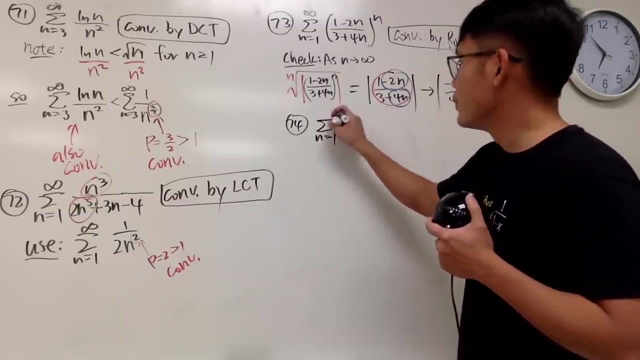 And you end up with one half Like that. So the root test- This right here is good, This right here- tells us It converges by the Root test, Just like that. So that's the idea. Now, Seventy four, Okay, The sum as n goes from One to infinity. 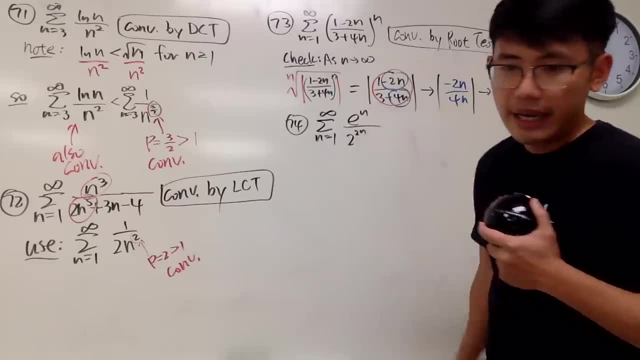 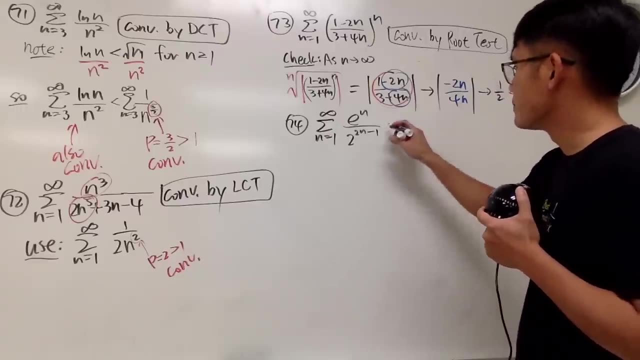 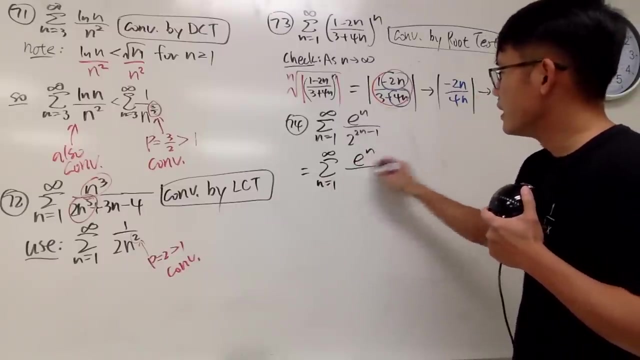 E to the n And minus one. So we have this, And perhaps we'll simplify this a little bit Before we do anything else. So here we go. This right here is the sum As n goes from one to infinity, And this is e to the n. Now let's do two things. 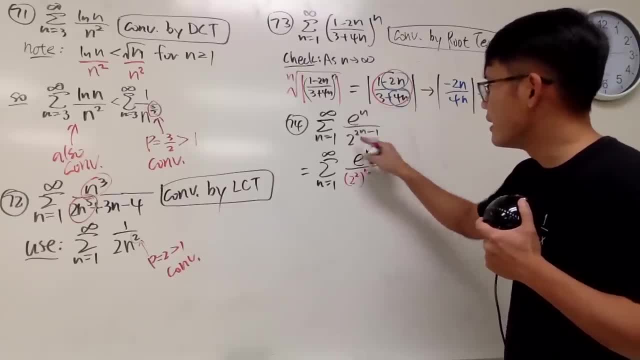 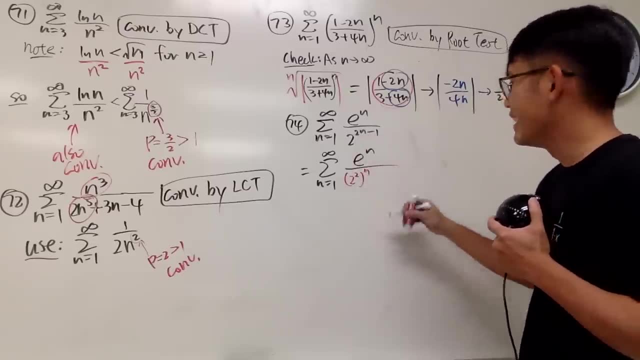 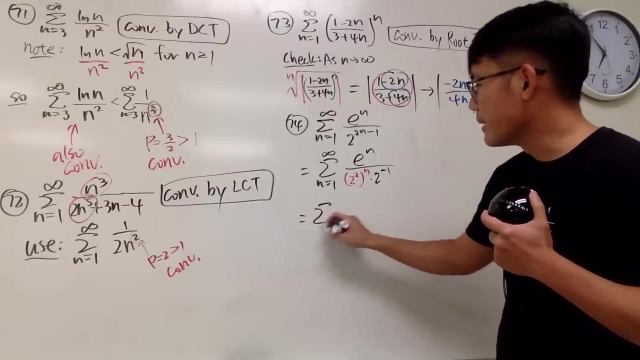 This part is the same as saying Two to the two and then n, Because you multiply the powers. You can just write two to the Power here and then Another power outside, And then the minus one means You multiply by two to the negative one, Like this. So now this right here is the sum. 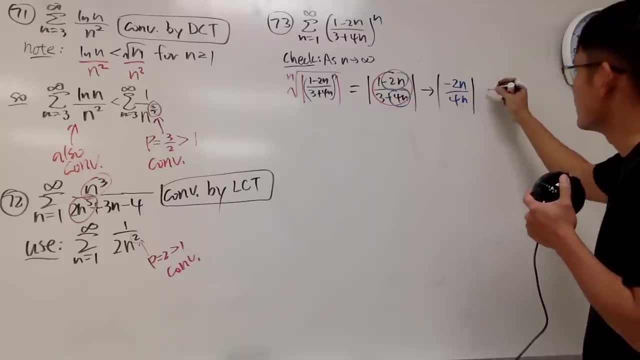 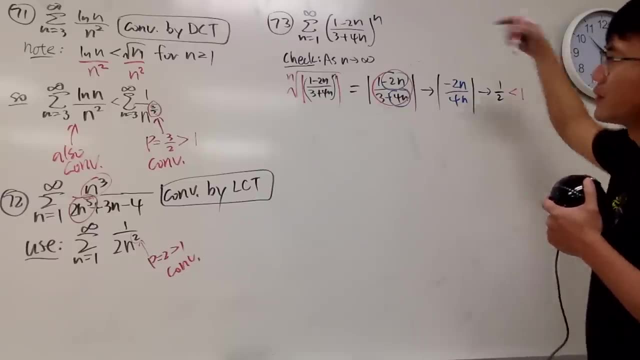 The absolute value is a continuous function, so you can just pretty much do that, and then you end up with 1 half like that, And of course it's less than 1 for the root test. This right here is good. 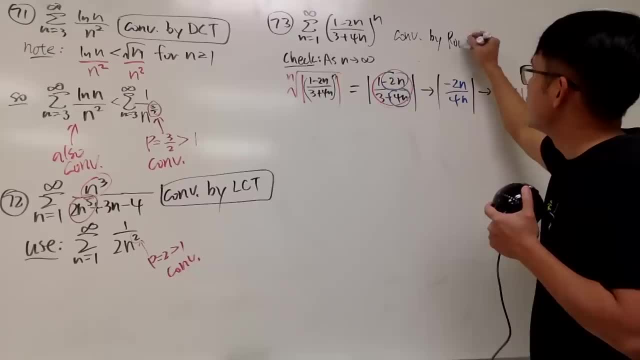 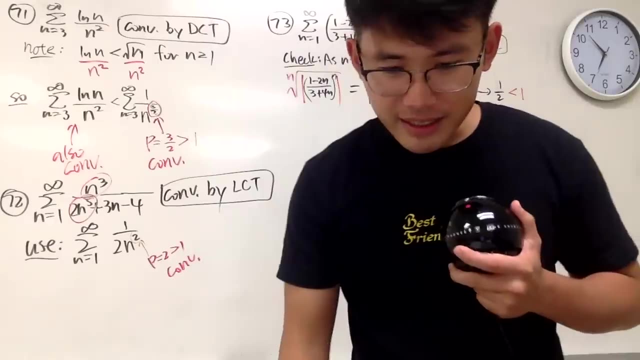 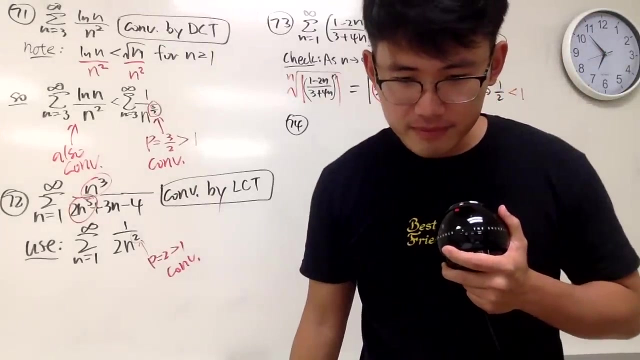 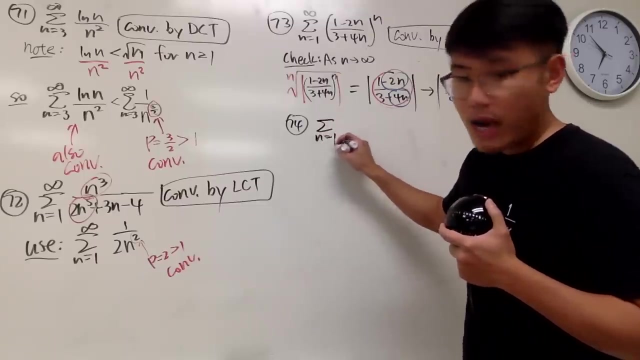 This right here tells us it converges by the root test. right, Just like that. So that's the idea. Now, 74. Okay, okay, okay. The sum as n goes from 1 to infinity, e to the n, over, 2 to the 2n and minus 1.. 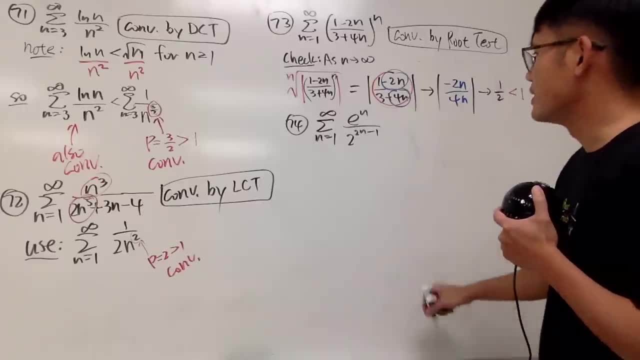 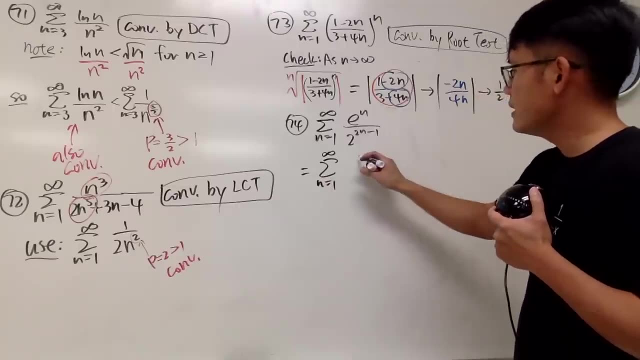 So we have this, And perhaps we'll simplify this a little bit before we do anything else. So here we go. This right here is the sum, as n goes from 1 to infinity, And this is e to the n. Now let's do two things. 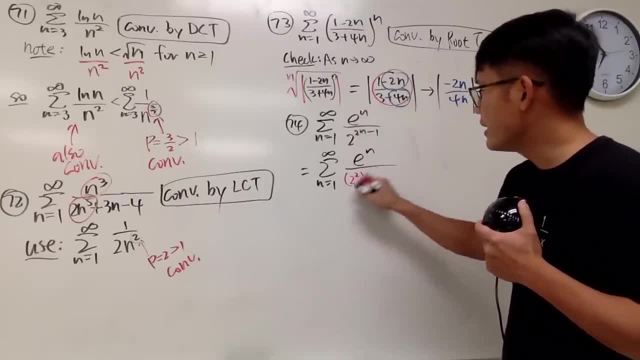 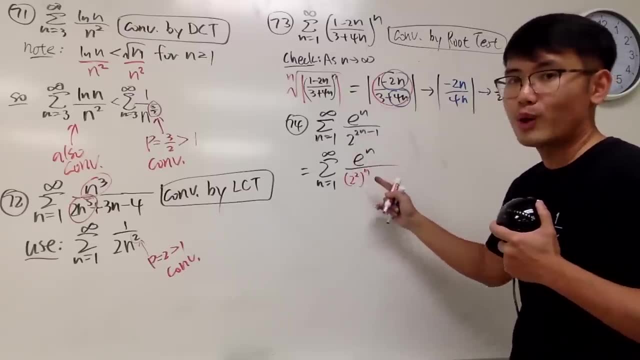 This part is the same as saying 2 to the 2 and then n, Because you multiply the powers. You can just write 2 to the power here and then another power outside, And then, don't forget, the minus 1 means you multiply by 2 to the negative 1, like this: 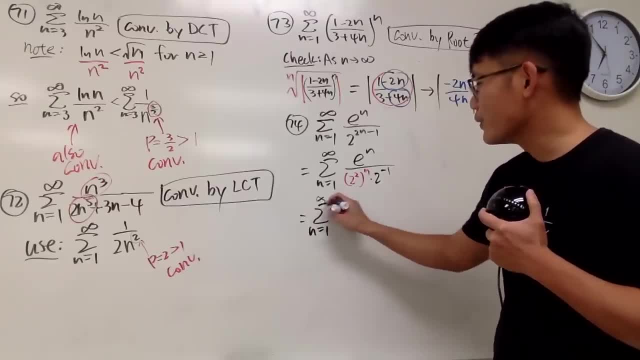 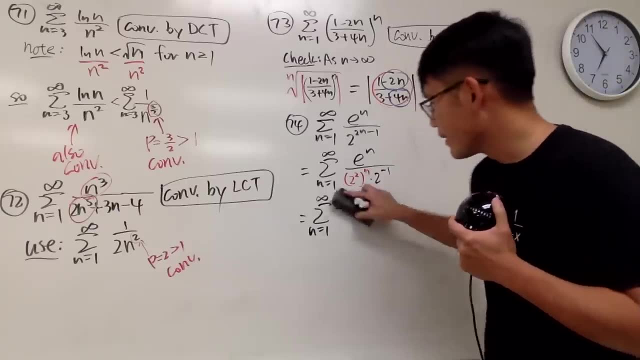 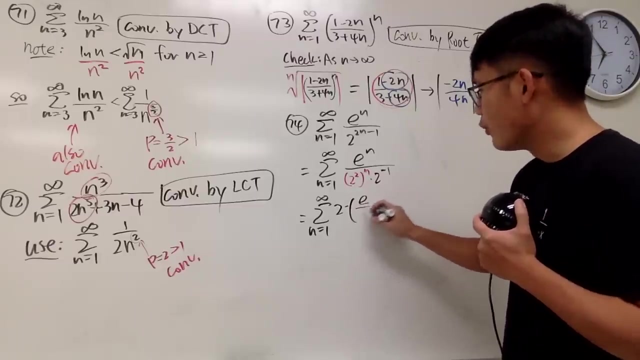 So now this right here is the sum as n goes from 1 to infinity. This right here can be brought up to become just a 2.. And we have e to the n over 4 to the n, So we can just multiply by e over 4 to the n, like this: 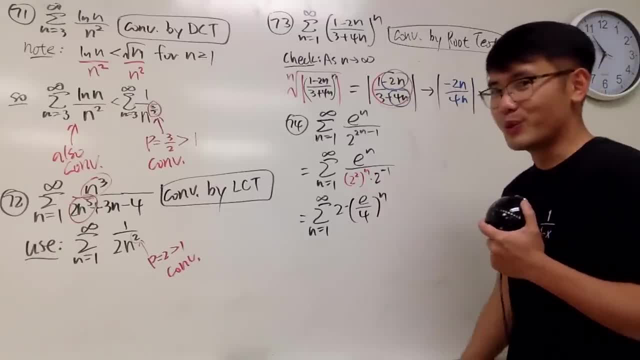 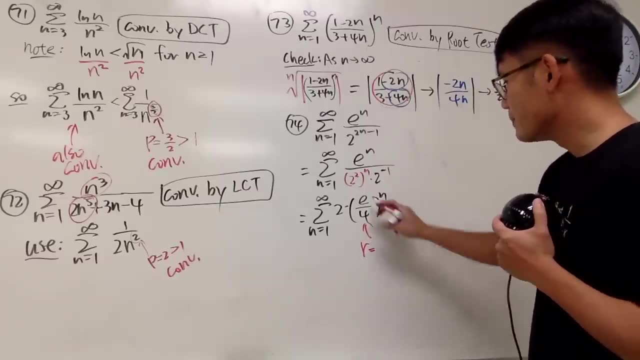 Now check this out. In fact, we can calculate the sum if we would like, right. But no, we don't need to, Because this right here is what. Yeah, r is equal to e over 4. And r is about. 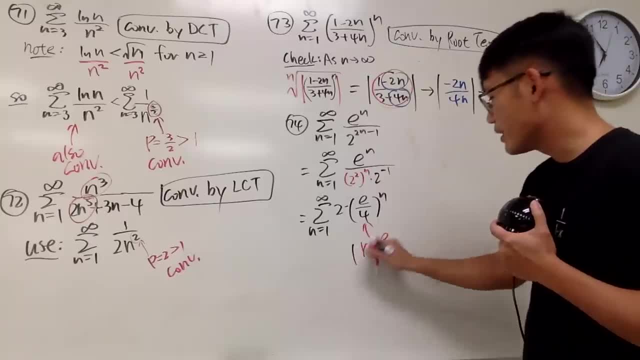 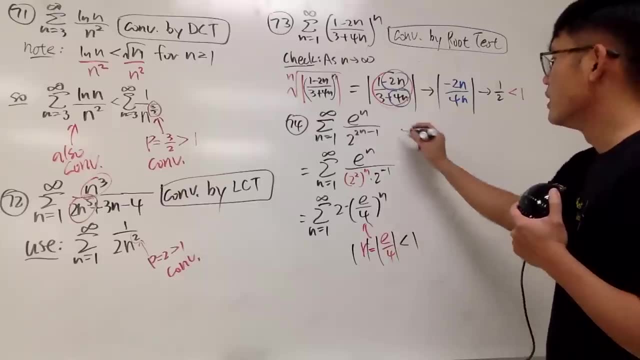 Oh sorry, e is about 2.7 something. So when we take the absolute value, this right here is less than 1.. So this is actually just a geometric series. Very nice right here. This right here converges by: 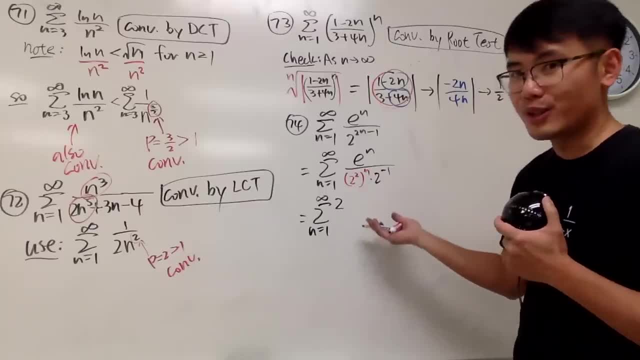 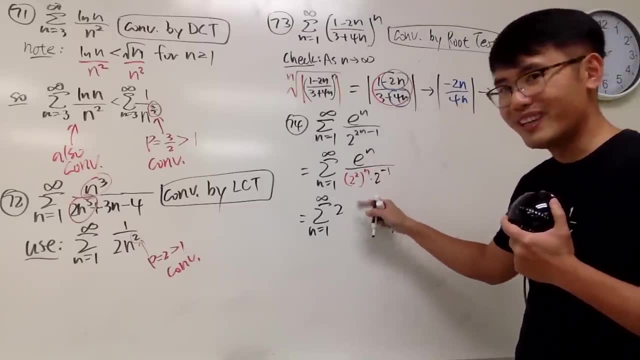 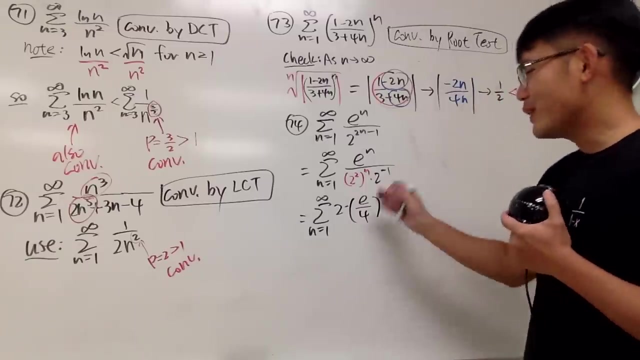 As n goes from one to infinity. This right here can be brought up To become just a two, And we have E to the n Over four to the n, So we can just multiply by E over four to the n, Like this. Now check this out. But no, we don't need to. 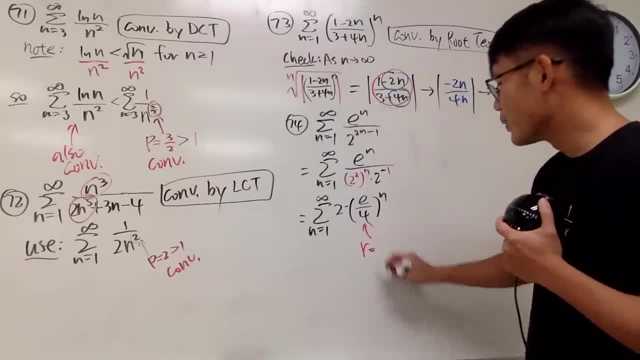 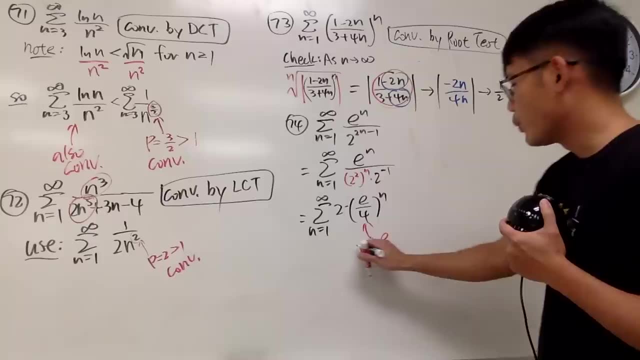 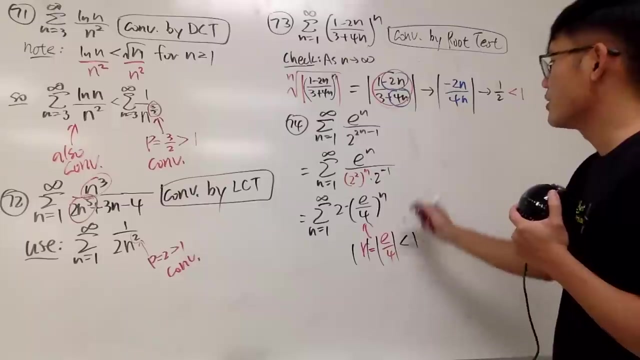 Because this right here is what R is equal to E over four, And R is about E is about 2.7 something. So when we take the absolute value, This right here is less than one. So this is actually just a geometric series. Very nice right here. 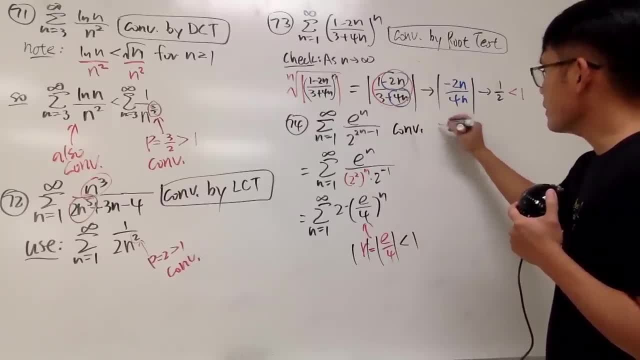 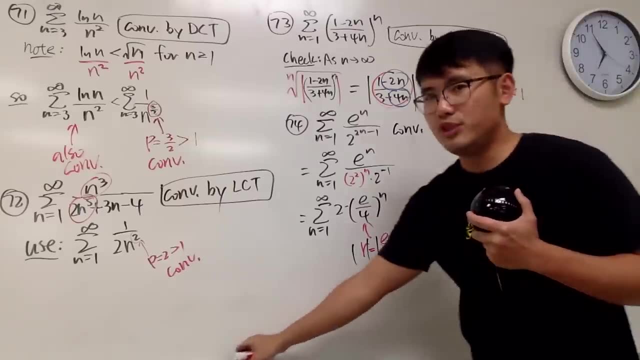 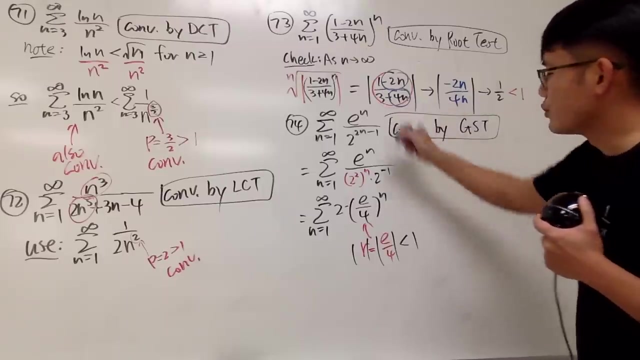 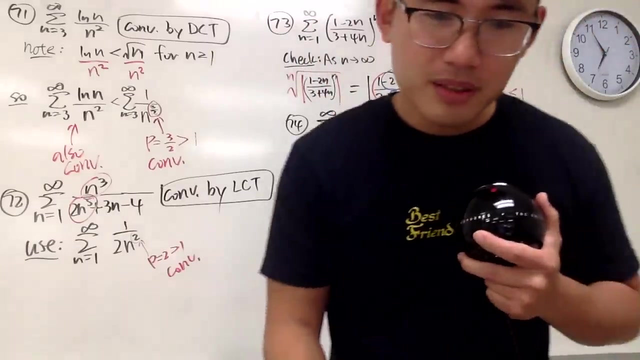 This right here converges By Well. first time By geometric, I would say, Geometric series test, GST, GST, Usually geometric, Just some like little thing that we We do to help us out To do the computer, But this time It's helping us out. Alright, I know I didn't do this for you. 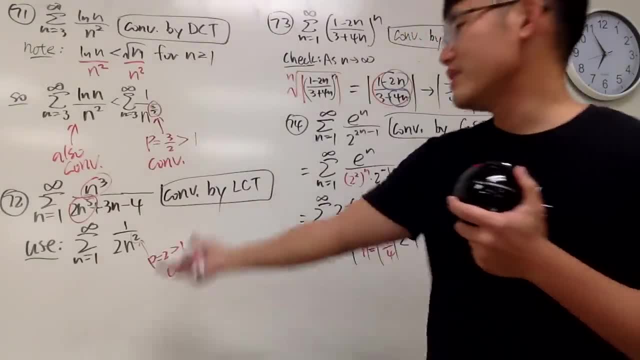 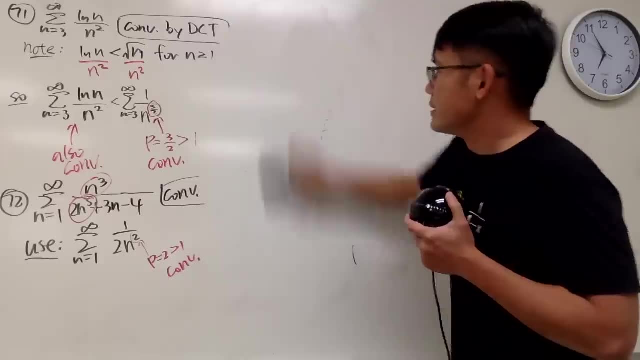 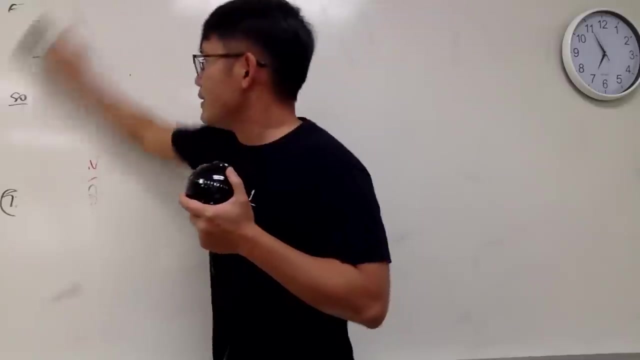 But I will do the next one for you guys. Well, I did Tell you guys how to do it, So, seriously, practice some of them. Alright, I want to see If I can go home by eight. I don't know. Well, I want to To go see my girlfriend by eight. 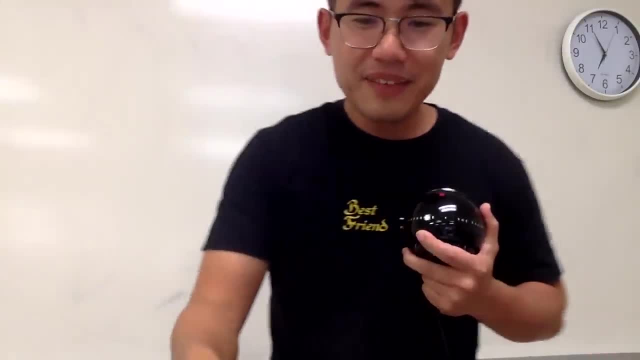 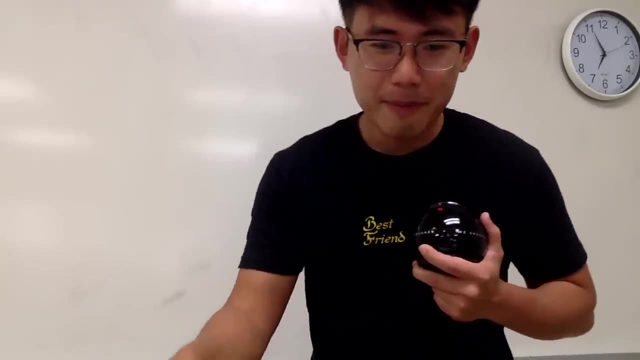 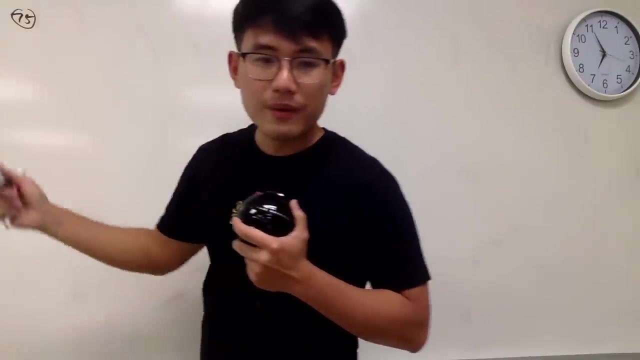 I will see. I will see. This is like It's definitely going to be longer than The integral test. I don't know. actually it's 430 right now. We'll see. It's a very nice comparison. Anyway. 75, The sum As n goes from one to infinity. 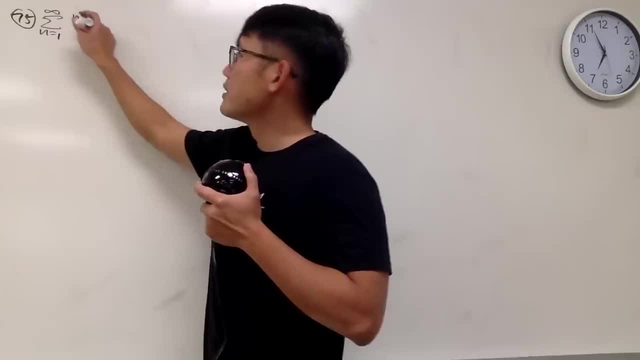 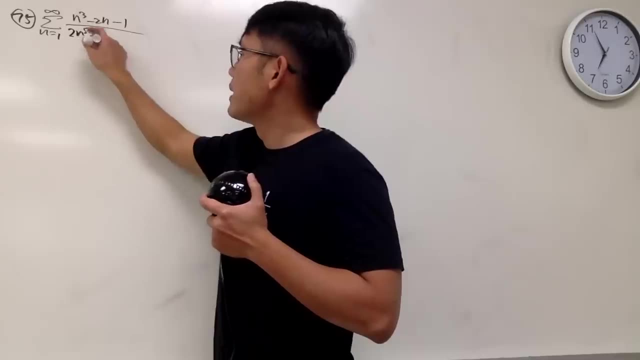 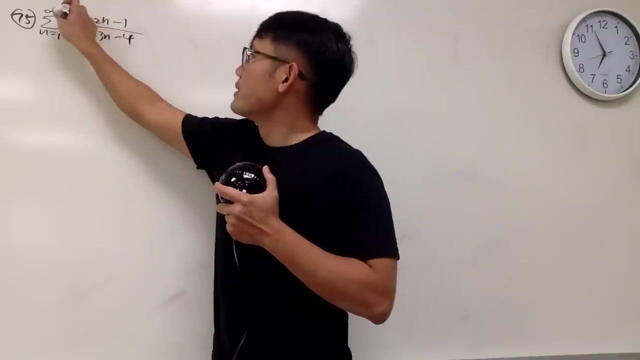 And then we have all the Crazy expression: n to the third power, Minus 2n, minus one, Over 2n to the five, Plus 3n minus four. You guys can see earlier I didn't do that, but I will do this for you. Okay, here we go. comparison: 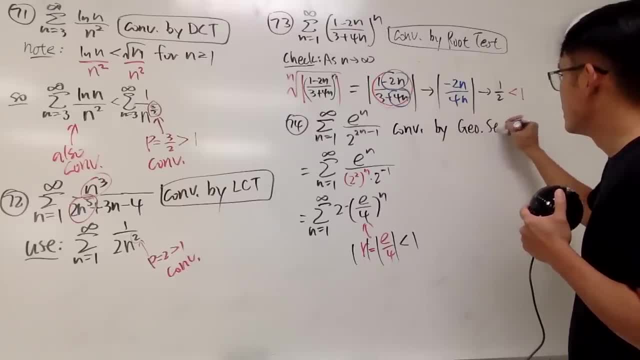 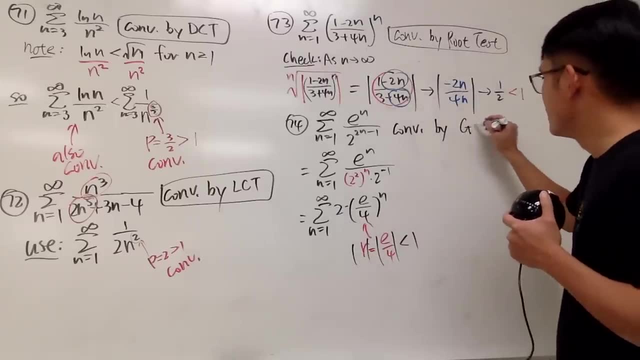 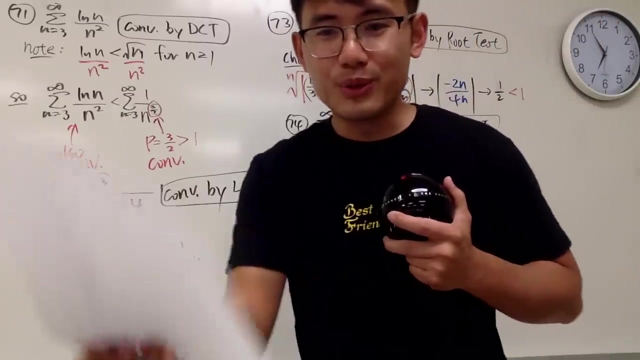 Well, first time right By geometric. I would say it's a geometric series test GST. Usually, geometric is just some little thing that we do to help us out to do the computer stuff, But this time it's helping us out. 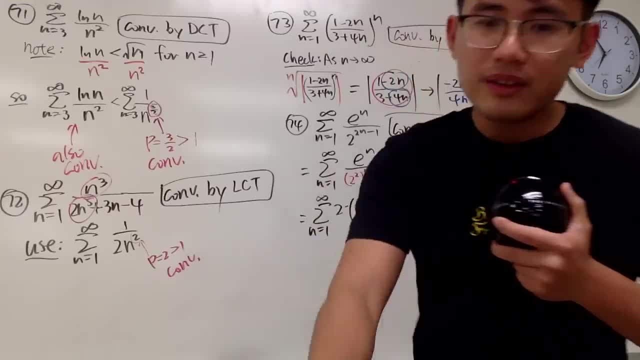 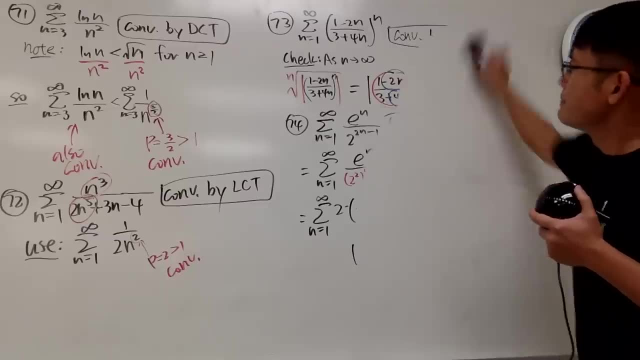 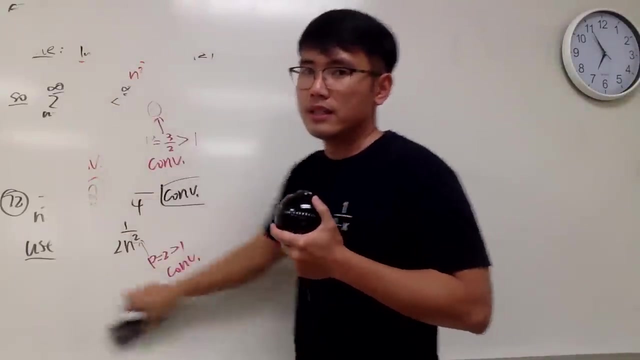 All right, I know I didn't do this for you, But I will do the next one, This one for you guys. Well, I did tell you guys how to do it. So, seriously, practice some of them. All right, I want to see if I can go home by 8.. 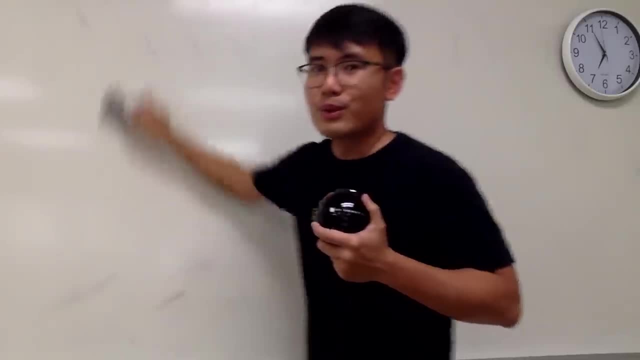 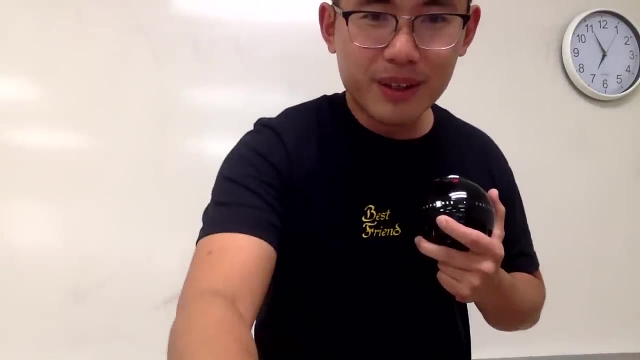 I don't know. Well, I want to go see my girlfriend by 8.. I will see, I will see, I will see. This is like It's definitely going to be longer than the integral test. I don't know. 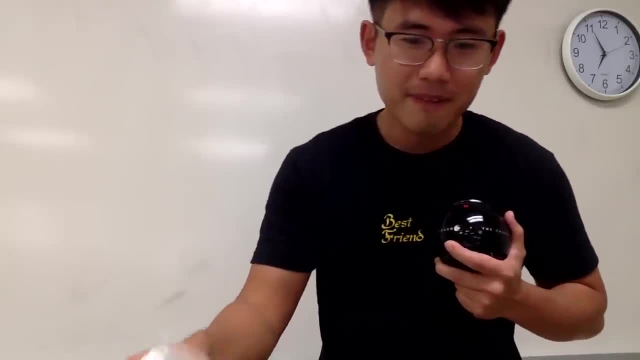 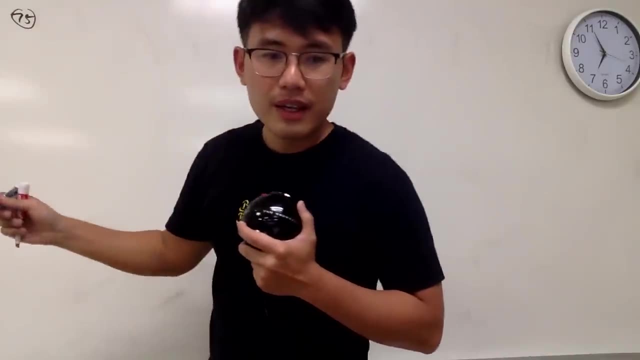 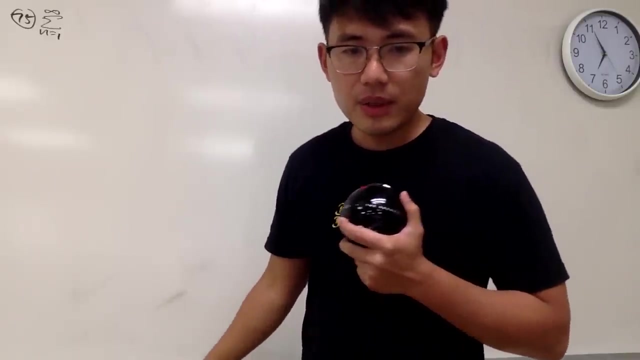 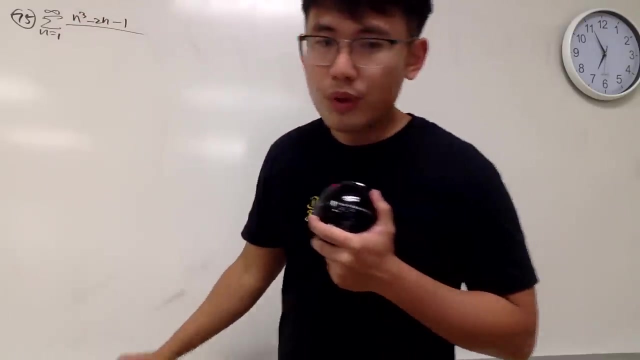 Actually it's 4.30 right now. We'll see. It's a very nice comparison. Anyway, 75 right here. The sum as n goes from 1 to infinity. And then we have all the crazy expressions: n to the third power minus 2n minus 1 over 2n to the 5 plus 3n minus 4.. 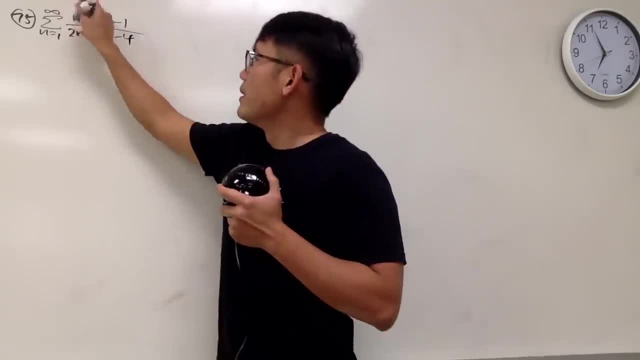 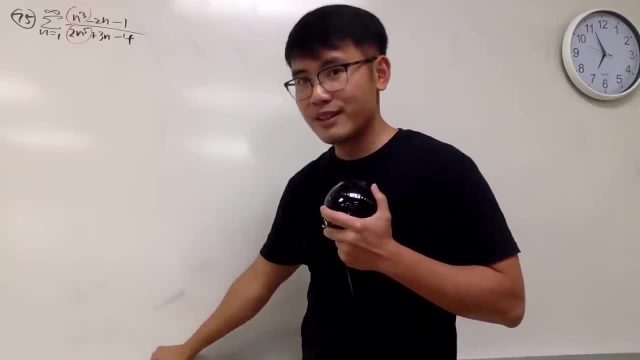 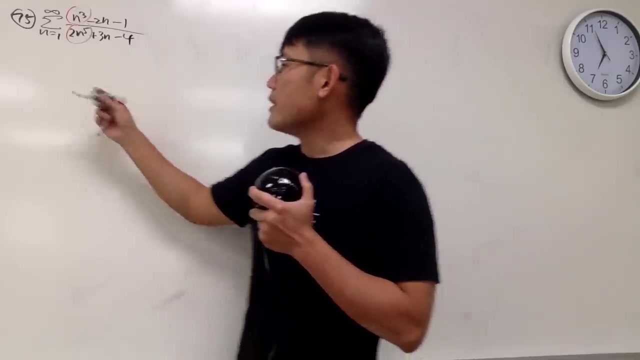 You can see, earlier I didn't do that, But I will do this for you. huh, OK, Here we go. Comparison: This and that, And let me just change to another marker, for the red one. Aha, Anyway, this is what we know, which is the sum as n goes from 1 to infinity. 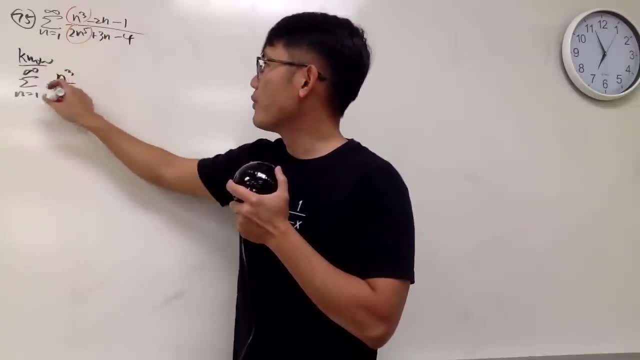 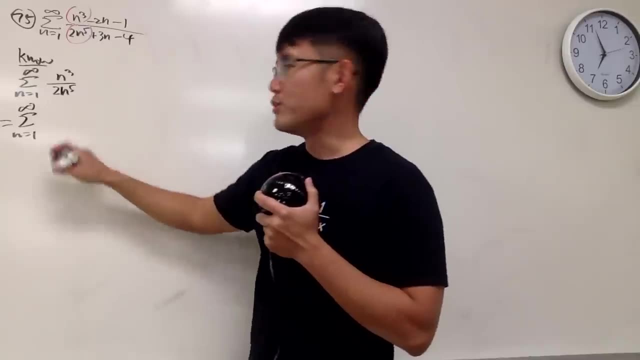 And we just have n to the third power over 2n to the 5. And of course this is the sum, as n goes from 1 to infinity. We can just do this real quick. This is 1 over 2n to the second power. 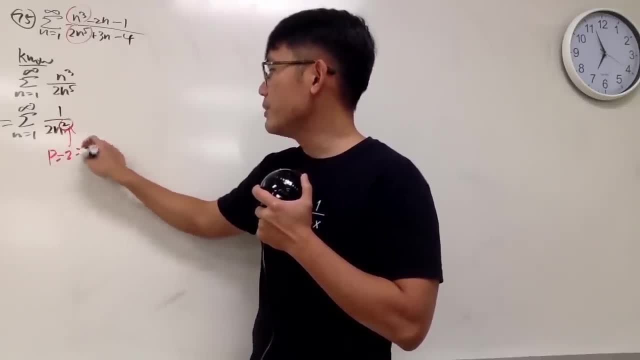 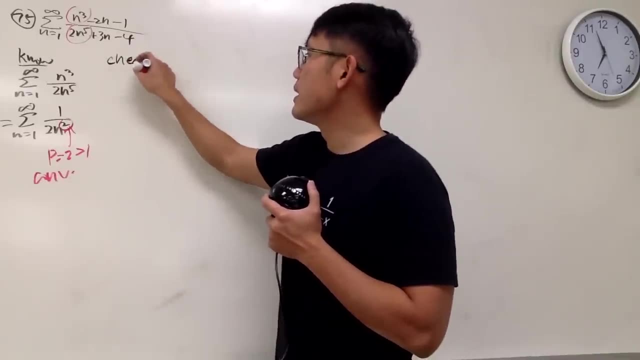 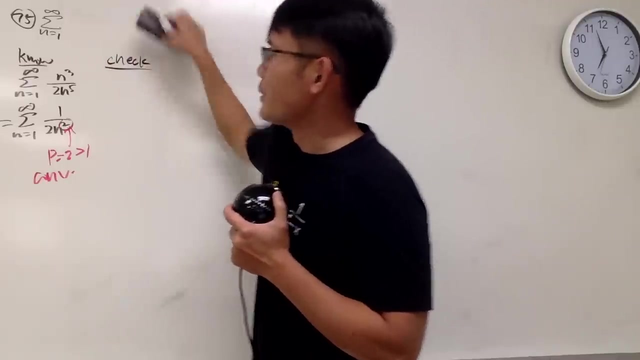 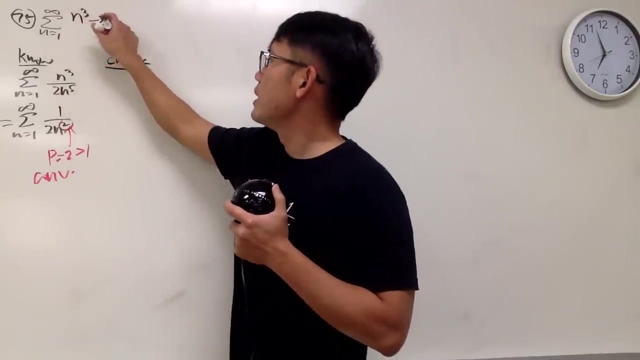 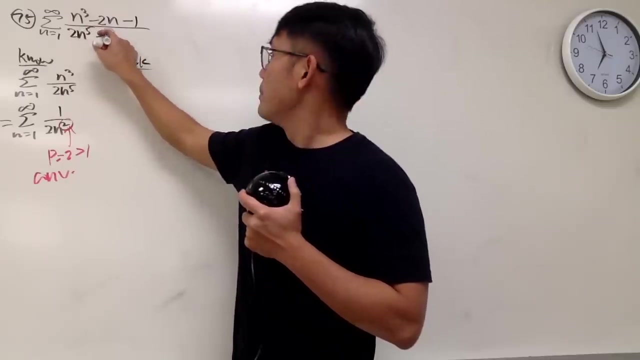 And this right here, p is 2,, which is bigger than 1,, which right here converges. Now let's do the check. Well, for the check, let me just rewrite the question better, I'm sorry. n to the third power, minus 2n, minus 1 over 2n to the 5, and then plus 3n, minus 4.. 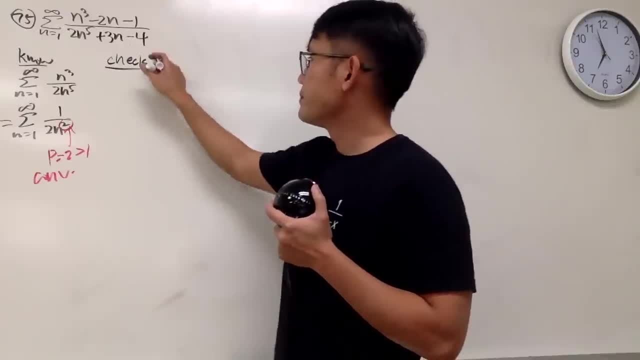 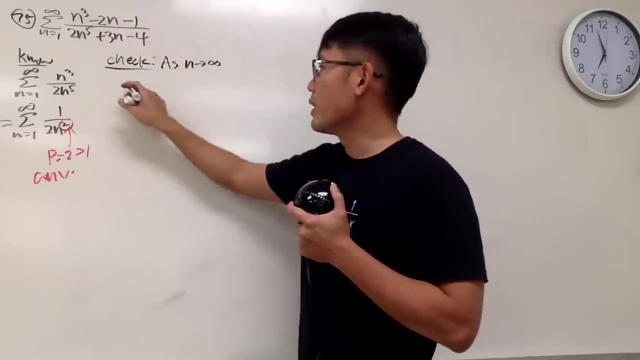 Like this Slightly better. All right Check. This is a limit comparison test And again, let me just put it: as n goes to infinity, Put down the one that we want on the top, which is n cubed minus 2n minus 1.. 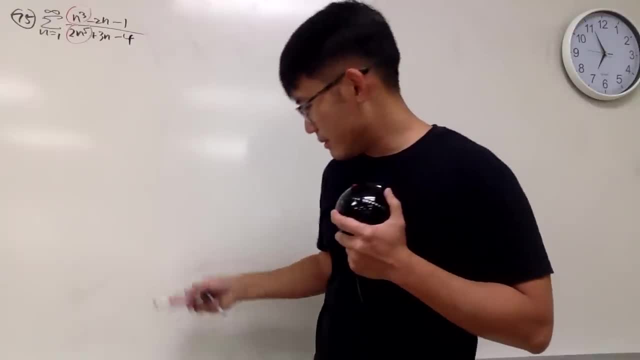 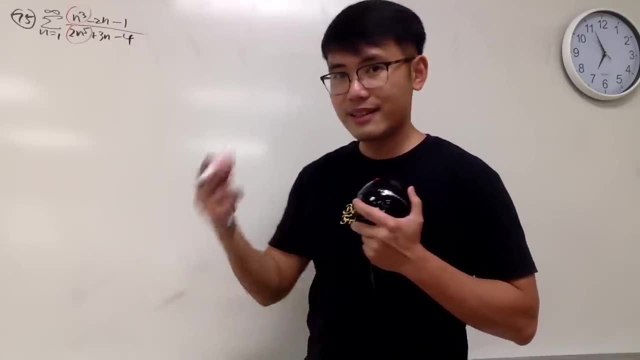 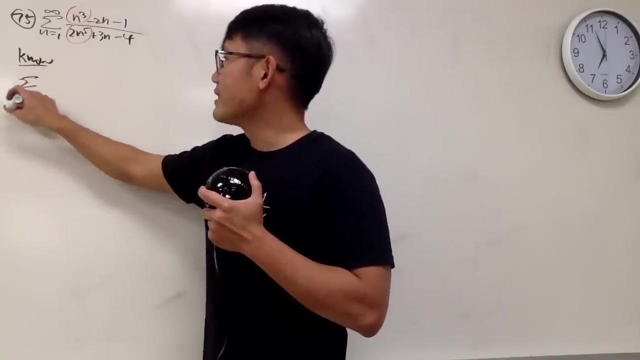 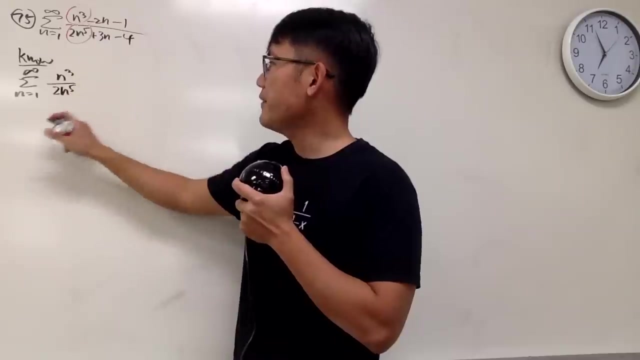 This and that, And let me just Change to another marker For the red one. Haha. Anyway, This is what we know, Which is The sum As n goes from one to infinity And we just have n to the third power over 2n to the five And, of course, this is the sum. 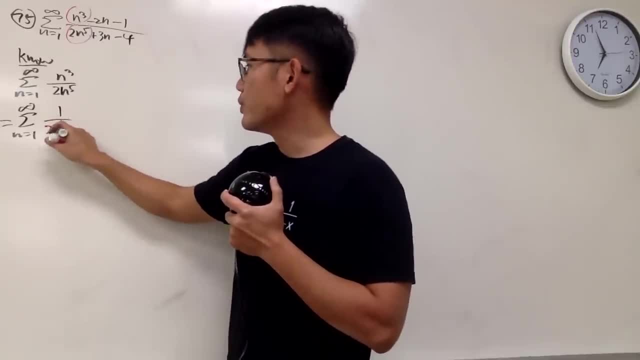 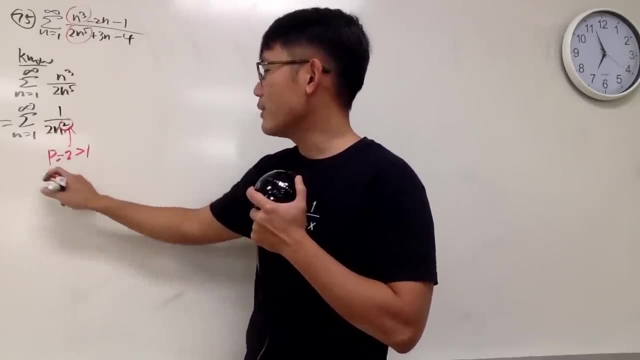 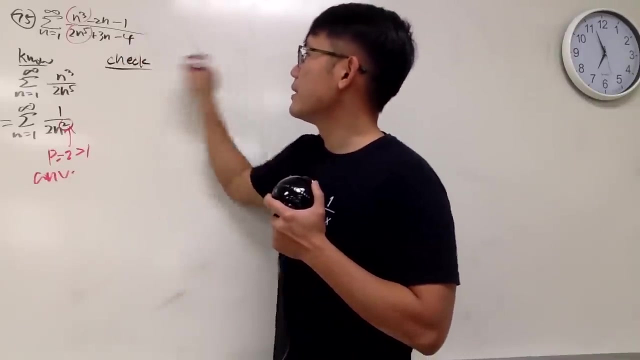 As n goes from one to infinity. We can just do this real quick. This is one over 2n. to the second power, P is two, Which is bigger than one, Which right here converges. Now let's do the check. Well, for the check, Let me just rewrite the question. 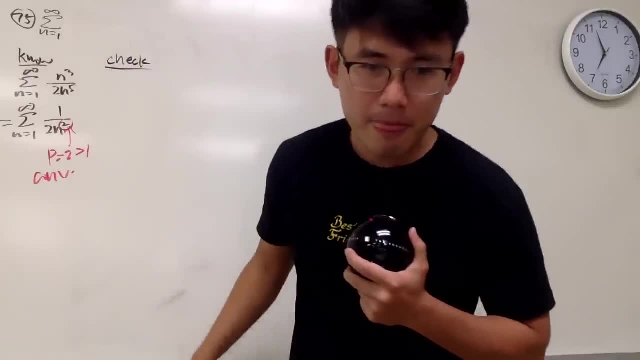 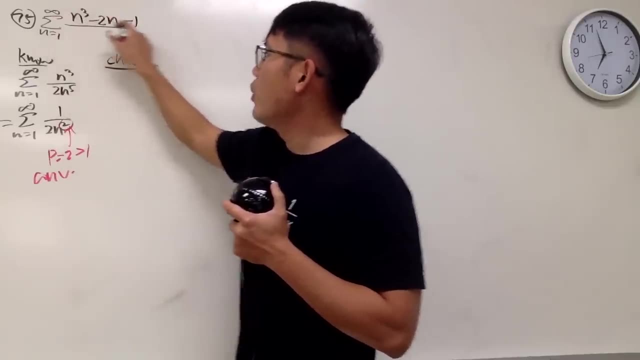 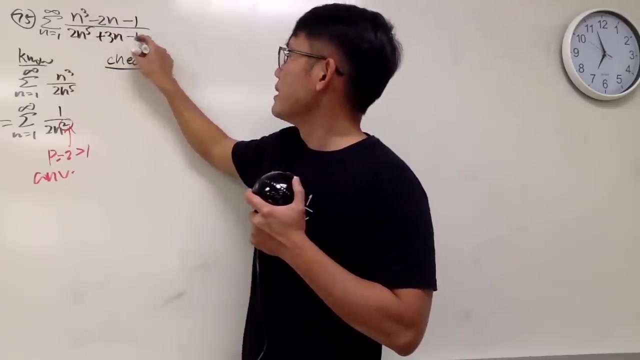 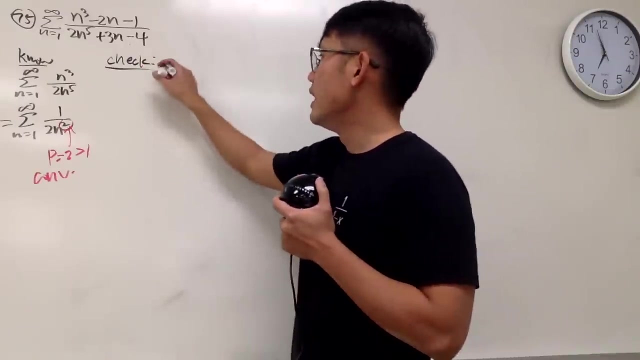 Better, I'm sorry. n to the third power, Minus 2n, Minus one Over 2n to the five, And then Plus 3n minus four, Like this slightly better. Alright, check. This is the limit comparison test. And again, let me just put it as: 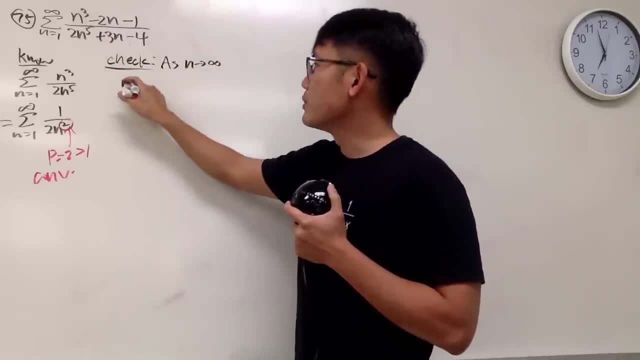 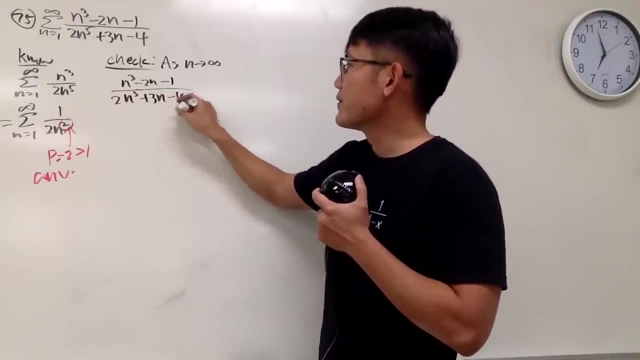 n goes to infinity. Put down the one that we want on the top, Which is n cubed minus 2n minus one Over 2n to the five plus 3n Minus four, And we will divide this by That guy, which is one over. 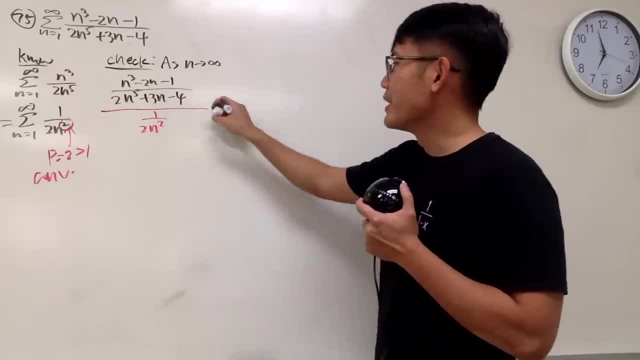 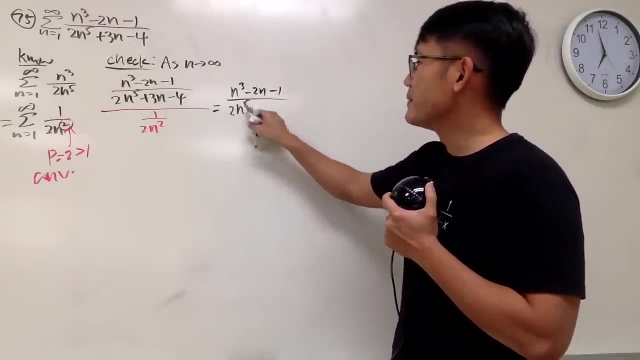 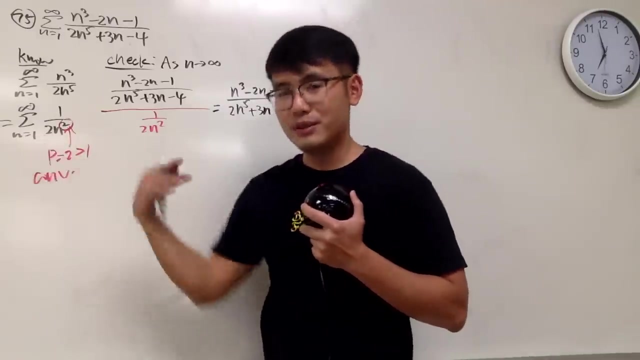 2n, to Take this flip that we get n cubed minus 2n minus one, Over 2n to the five Plus 3n minus four. And by the way, Even though I have this two right here, It's just a constant multiple, So it's still converging. 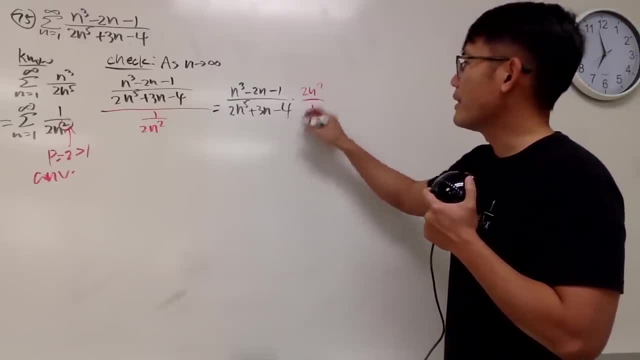 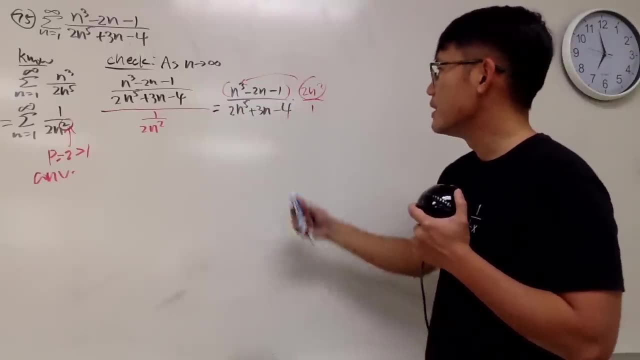 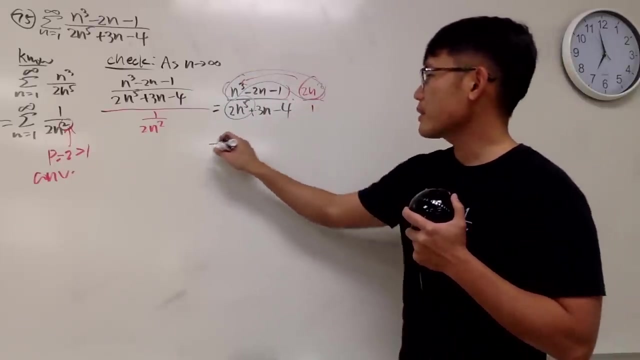 Alright, multiply by 2n, squared over one, Take this, distribute into all that And then, when you do that, You have the first term. So the truth is You pretty much consider these two guys And then this guy on the bottom. All in all They are Both with n to the fifth power. 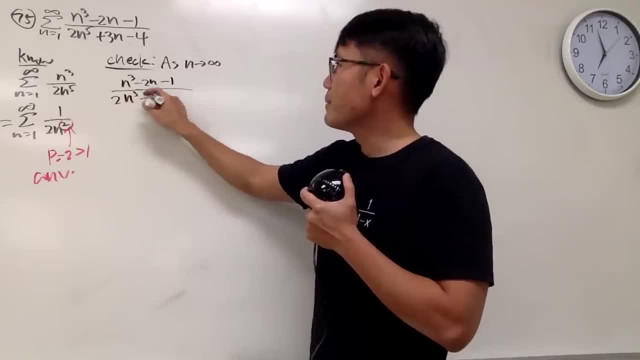 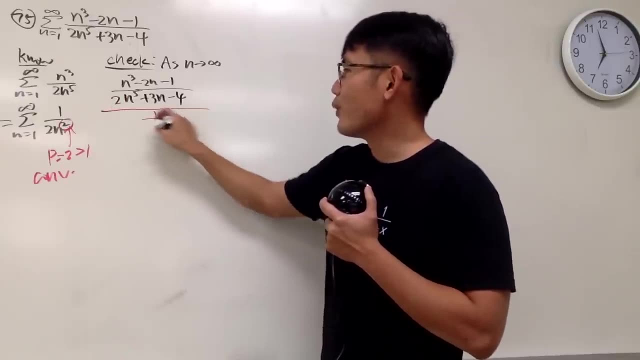 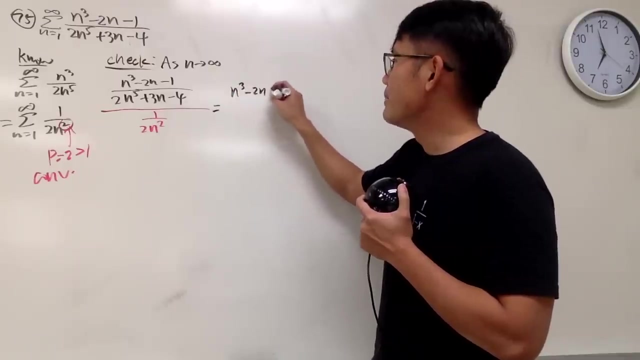 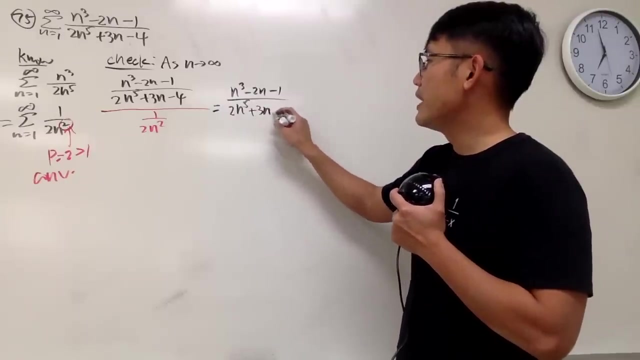 Over 2n to the 5 plus 3n minus 4.. And we will divide this by that guy, which is 1 over 2n to the 2.. Take this Flip that We get n cubed minus 2n minus 1 over 2n to the 5 plus 3n minus 4.. 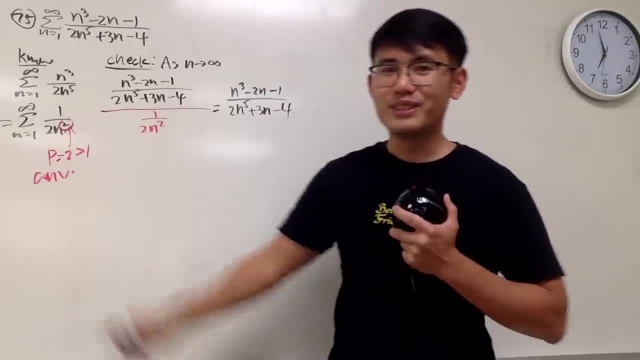 And, by the way, even though I have this 2 right here, it's just a constant multiple, So it's still converging. So anyway, just wanted to say: All right, Multiply by 2n squared over 1.. 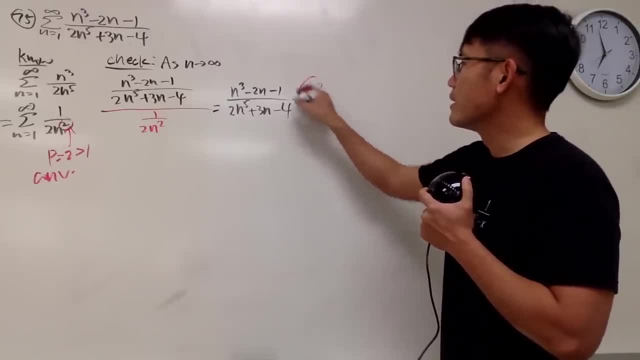 Take this, Distribute into all that And then, when you do that, you have the first term being the biggest that you have to consider. So the truth is, you pretty much consider these two guys and then this guy on the bottom. 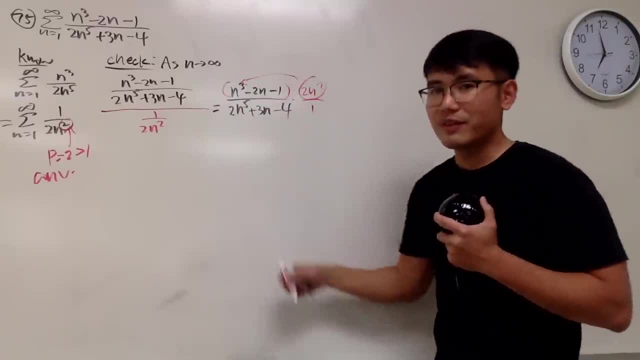 All in all they are, you know, both with n to the 5th, power and the coefficient are both equal to 2.. So you approach 1.. Now, let's look at the next one. Let's look at the next one. 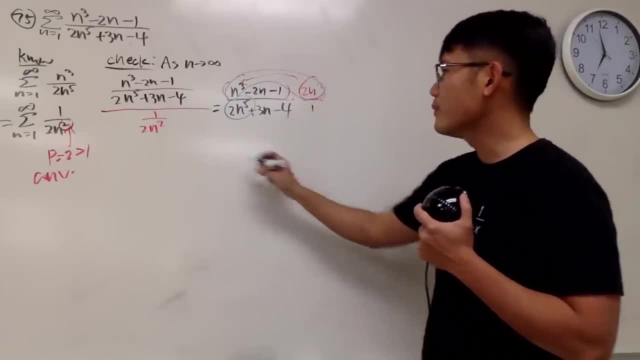 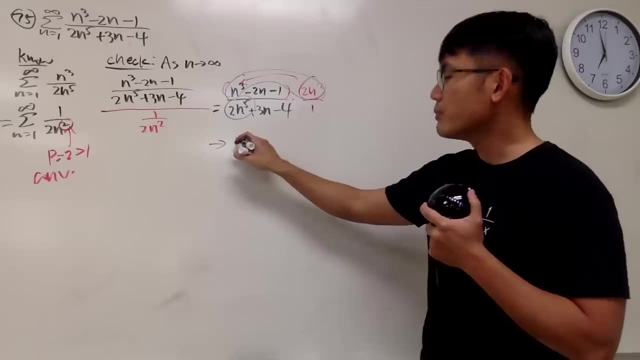 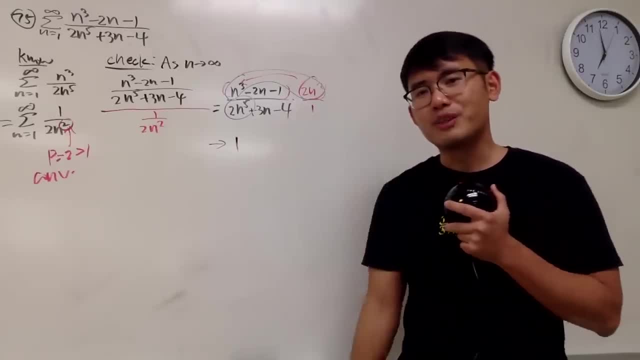 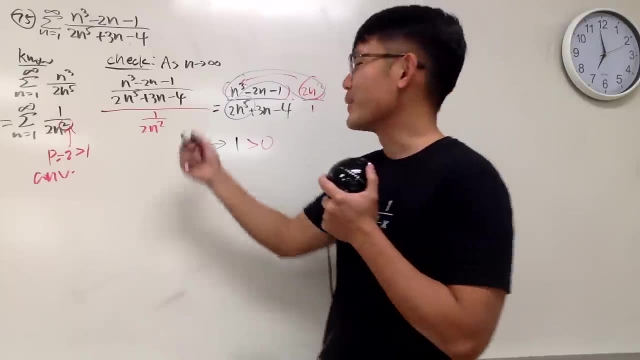 So you approach 1. This right here is the limit comparison test. As long as it's greater than 0, which it is- we can draw a conclusion. This and that have the same conclusion. So we know this right here converges. 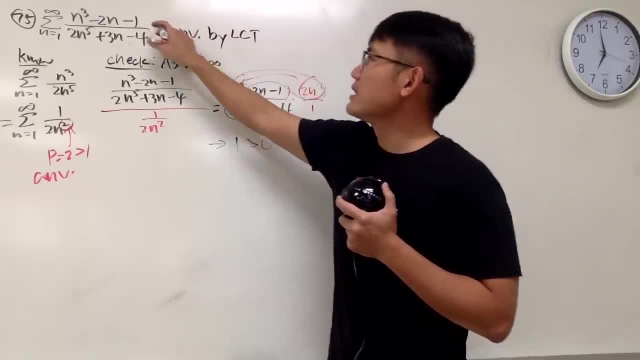 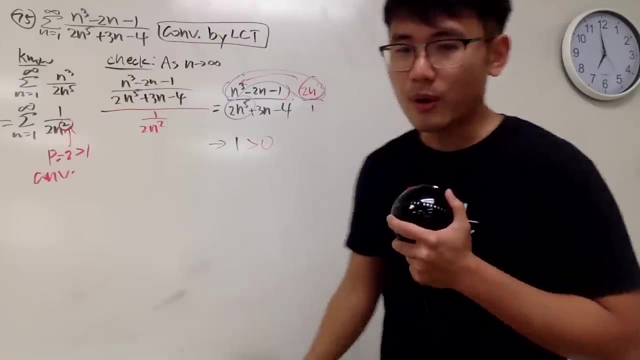 How come By the limit comparison test? And if you want to do an equality check, that would be slightly overkill. So limit comparison test will be the way to go. Number 76.. Okay, How are you guys doing? We're doing good, huh. 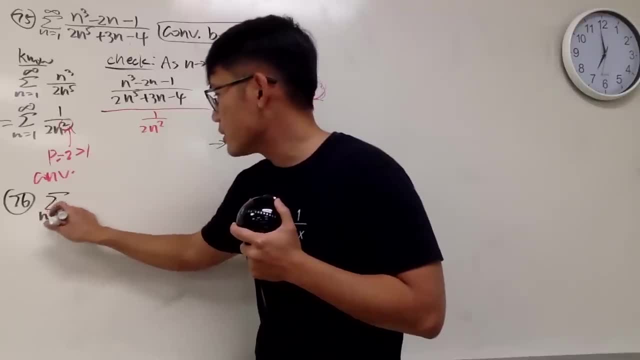 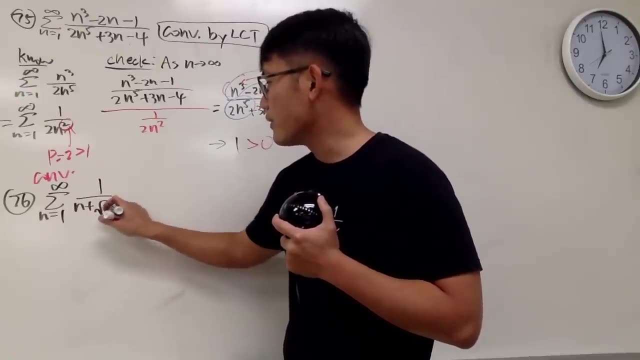 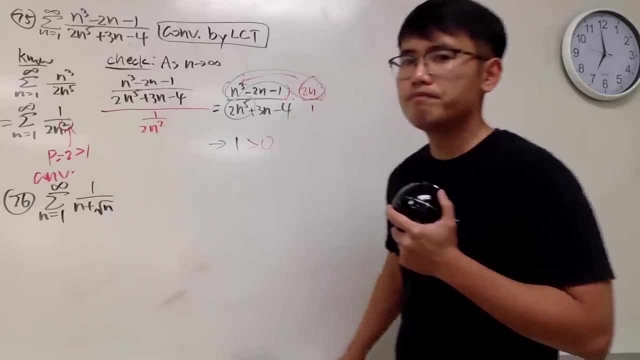 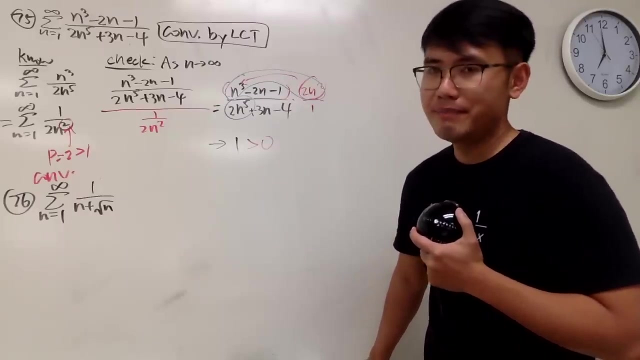 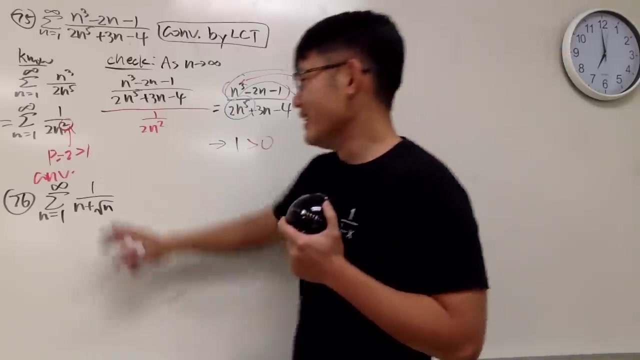 So, as n goes from 1 to infinity and we have 1 over n plus square root of n, like this, Most likely diverges Right. Most likely diverges Right. Most likely diverges. Why? Because we can just do this. 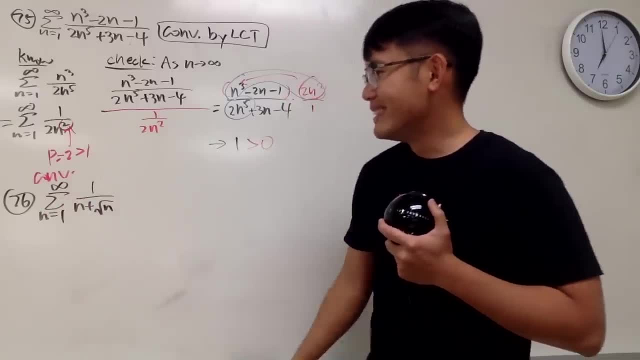 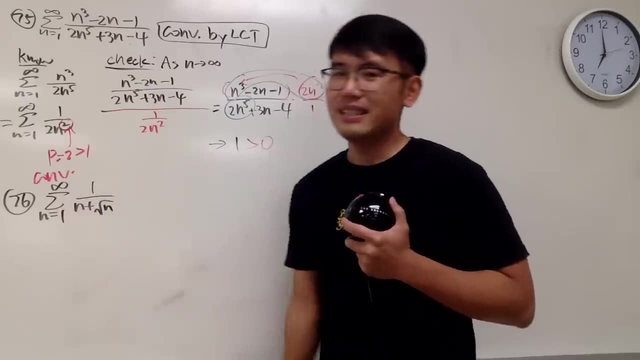 You can pick this guy or you can pick that guy. Up to you. If you want to do the limit comparison test, you have to pick the permutating part, which is this guy. If you pick this guy, not so much. 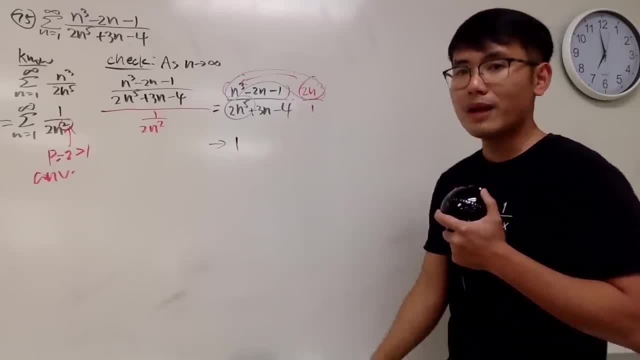 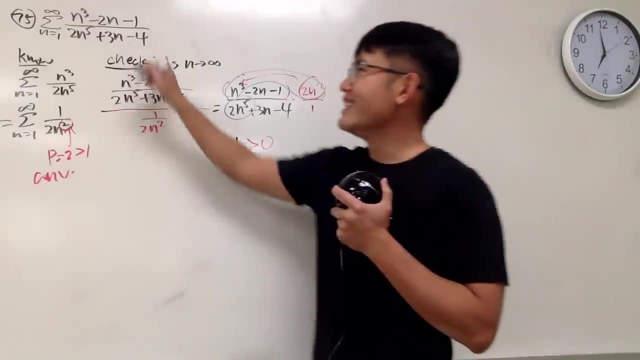 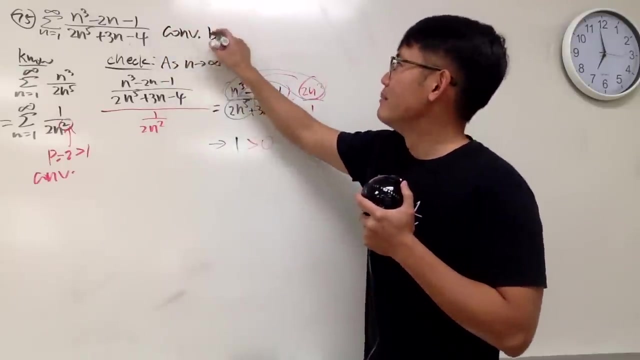 And the coefficient are both equal to two. So approach one. This right here is the limit comparison test. As long as it's Greater than zero, which it is, We can draw a conclusion. This and that have the same conclusion. So we know this right here converges. How come? 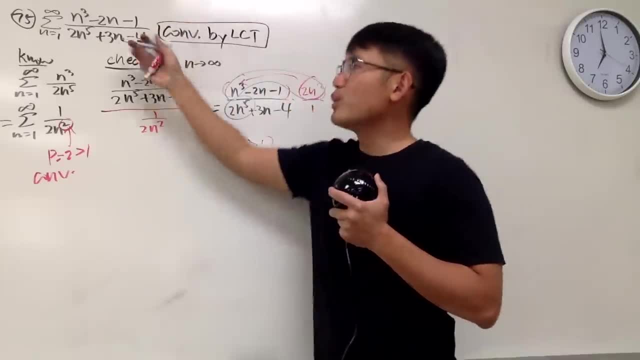 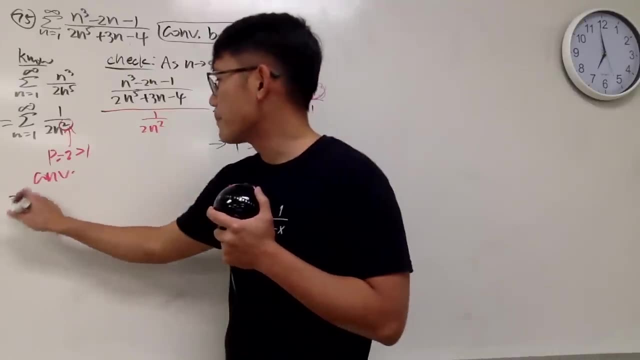 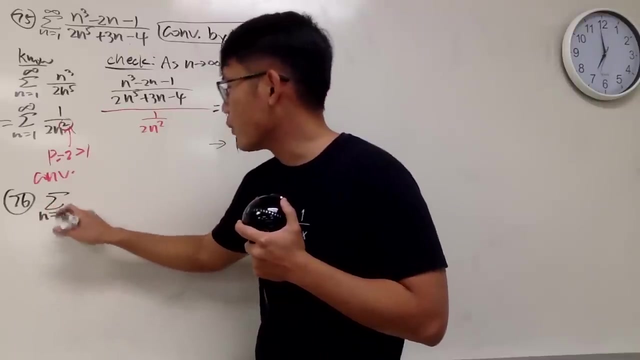 This is the limit comparison test, And if you want to do Inequality check, that will be Slightly overkill, so limit comparison test Will be the way to go. Number seventy six: Okay, how are you guys doing? We are doing good, huh. Sum as n goes from one. 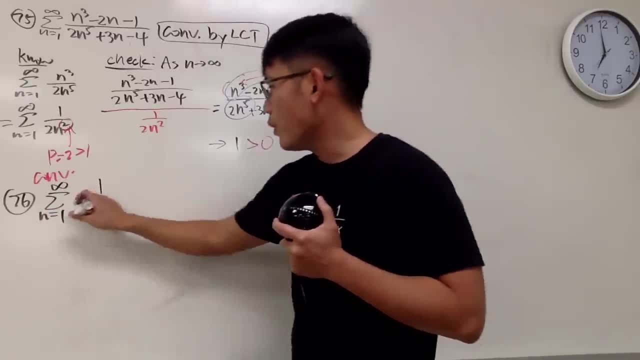 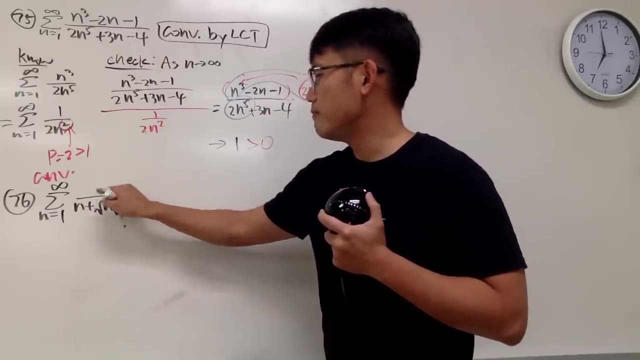 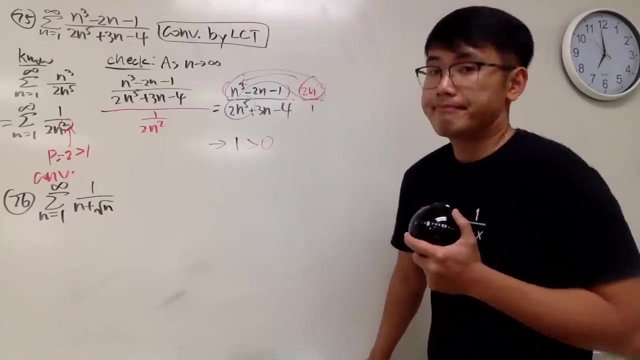 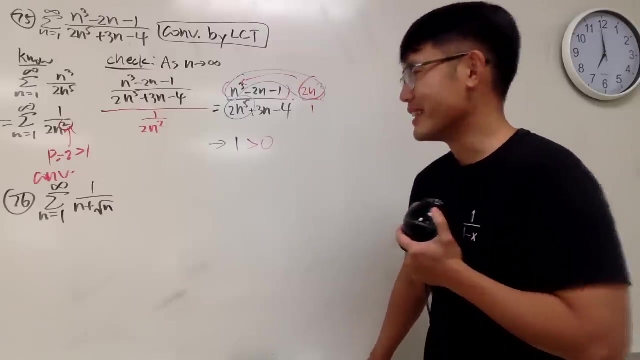 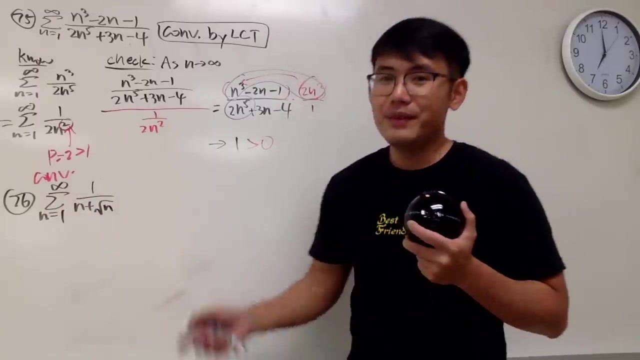 To infinity, And we have one over n plus square root of n, like this: Hmm, The total number Is The Number Most likely Diverges. Right, Most likely diverges. Why? because we just do this. You can pick this guy Or you can pick that guy, up to you. 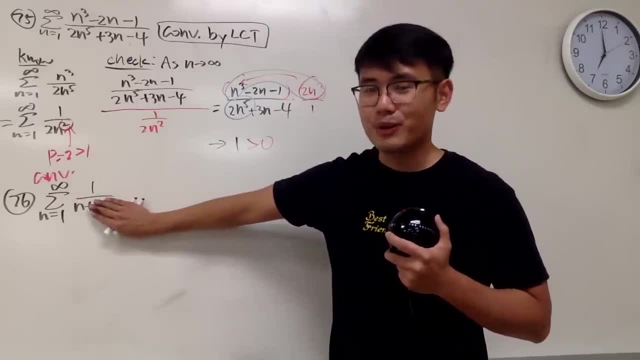 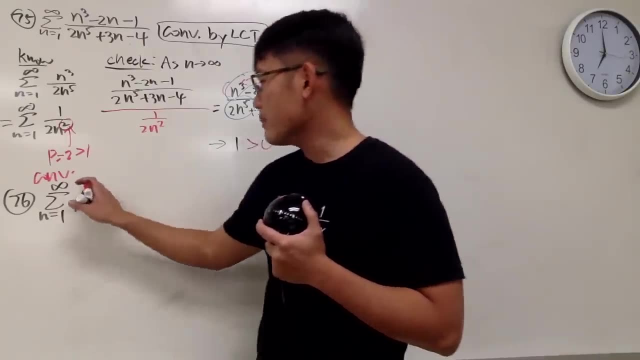 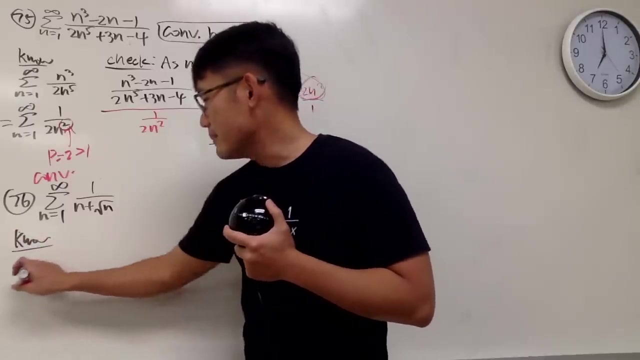 If you want to do the limit comparison test, You have to pick The dominating power, which is this guy. If you pick this guy, I'll take that back. So, anyway, pick this guy. So I'll just put this down right here. We know that the sum as n goes from 1 to infinity, 1 over n. 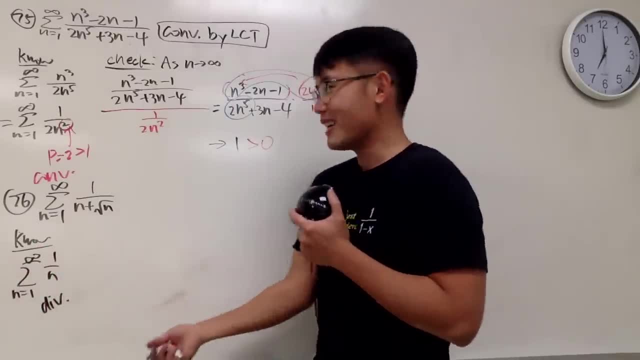 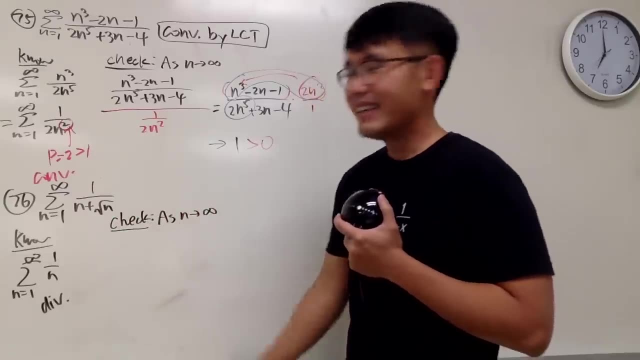 this right here diverges because we've been doing this so many times. And then again, let's go ahead and check the limit, as n goes to infinity. Here you get 1 over n, plus square root of n over 1 over n. 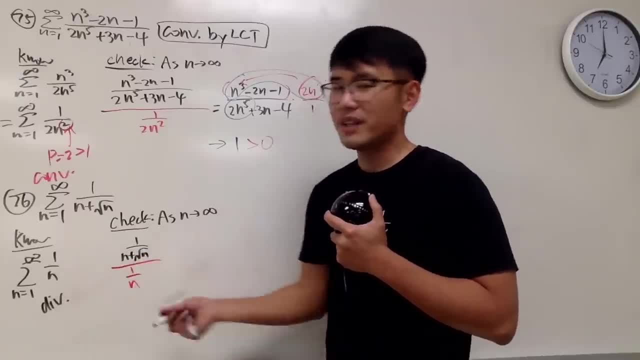 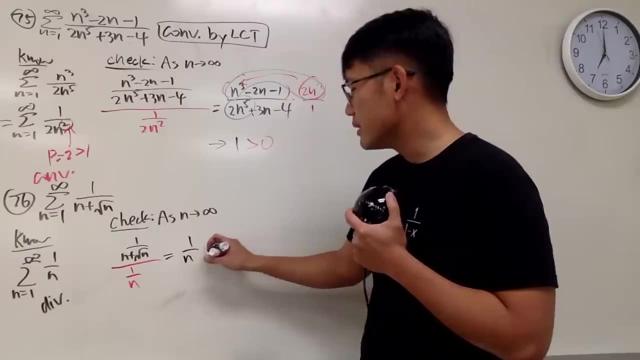 Again, you have to pick 1 over n right here. If you do a square root of n, it actually will give you 0, so that's bad Flip, that you get 1 over n, plus square root of n times n over 1.. 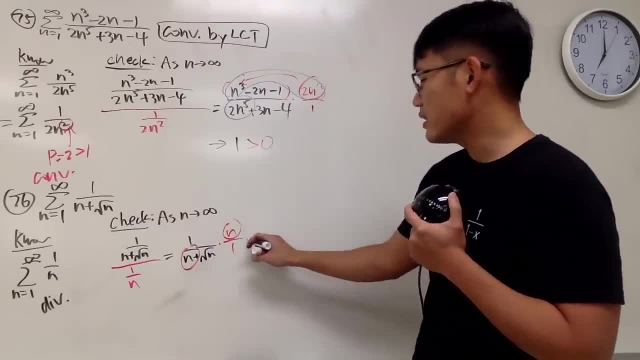 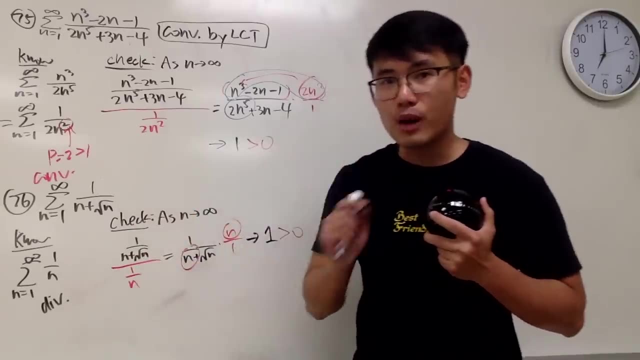 And you pretty much care about this. you care about that And again, similar to this idea, you will just get a limit being 1, and this, This right here, is greater than 0,, so we can come back here. They have the same conclusion. 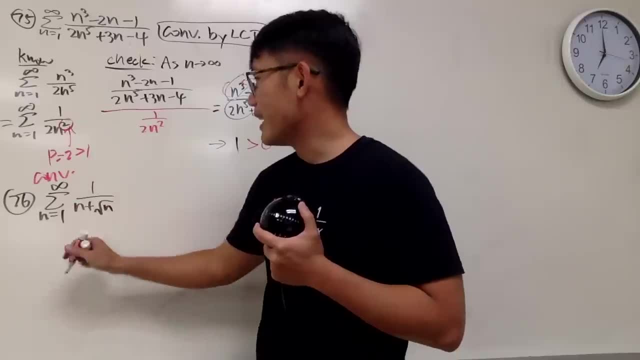 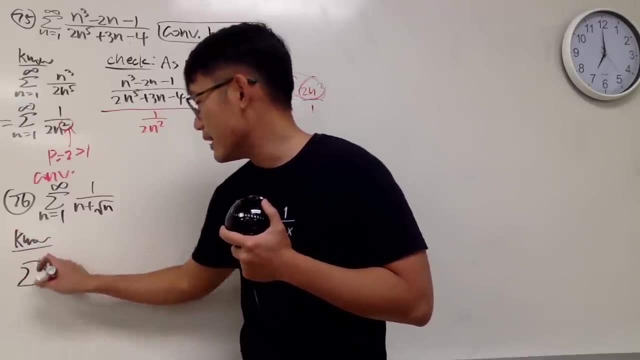 Not so much. I'll take that back. So, anyway, pick this guy. So I'll just put this down right here. We know that The sum Yes goes from 1 to infinity, 1 over n. This right here diverges. 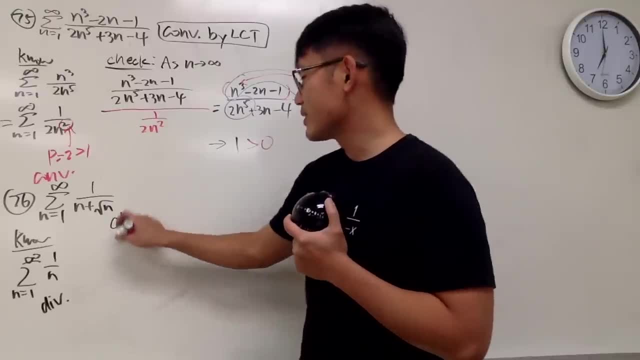 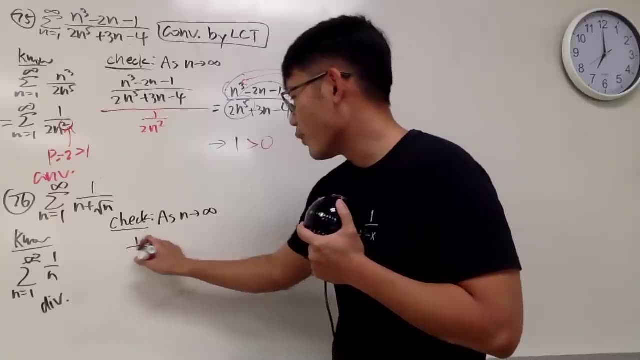 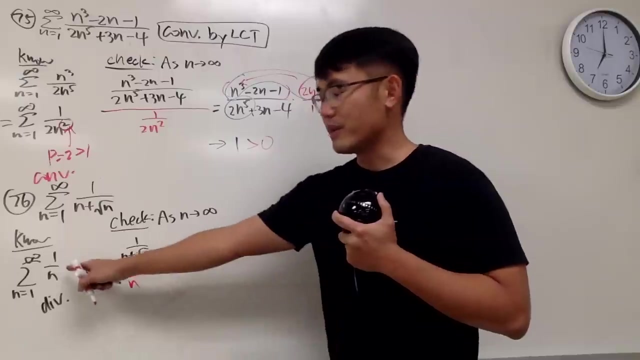 because we've been doing this so many times. And then again, let's go ahead and check the limit as n goes to infinity. Here you get 1 over n, plus square root of n over 1 over n. Again, you have to pick 1 over n, right here. 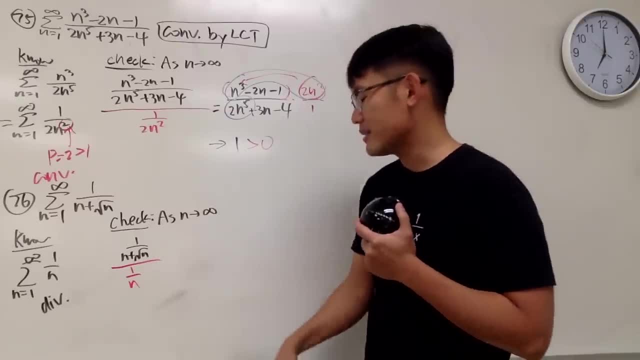 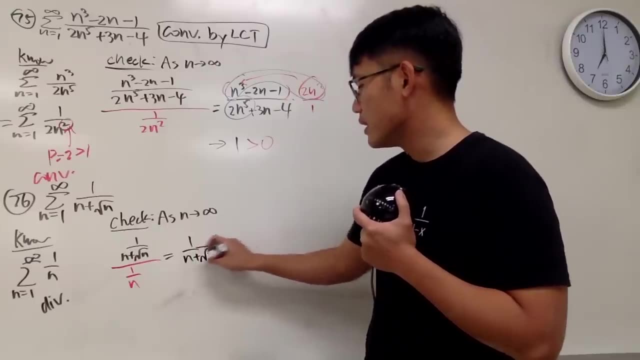 If you do a square root of n, it actually will give you 0, so that's bad Flip, that You get 1 over n, plus square root of n times n over 1.. And you pretty much care about this. you care about that. 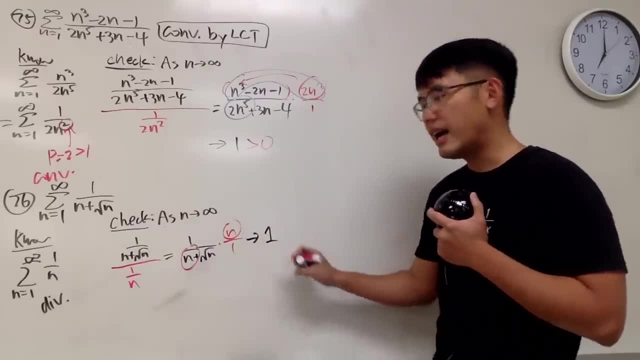 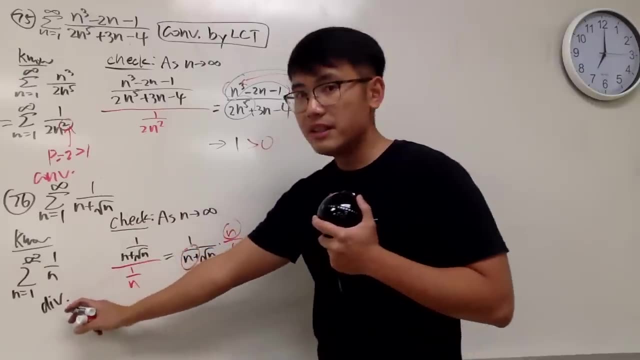 And again similar to this idea, you will just get a limit being 1, and this right here is greater than 0. So we can come back here. They have the same conclusion. So if this diverges, this right here also diverges. 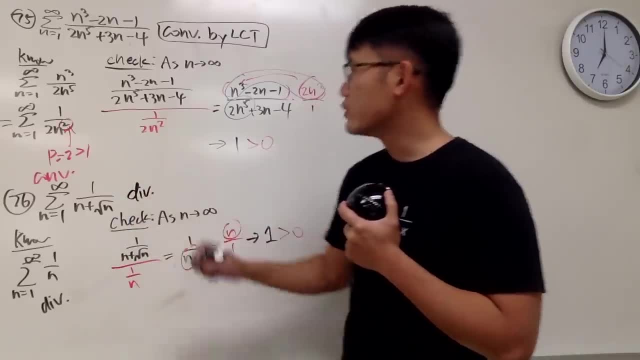 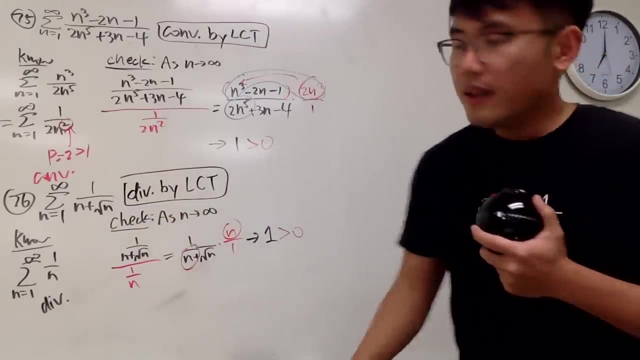 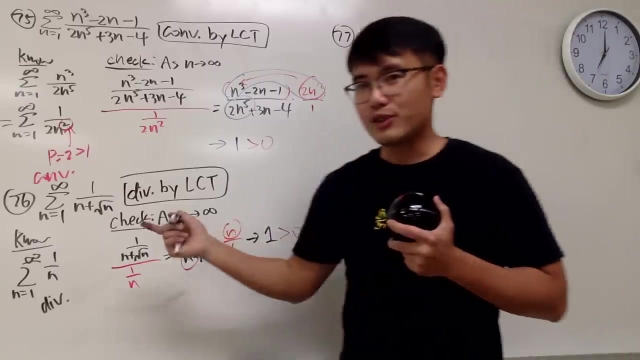 because they are about the same size. This right here diverges as well by the limit comparison test, like that Right Now. number 77. A slightly interesting one, Not really, No, it's actually really interesting. 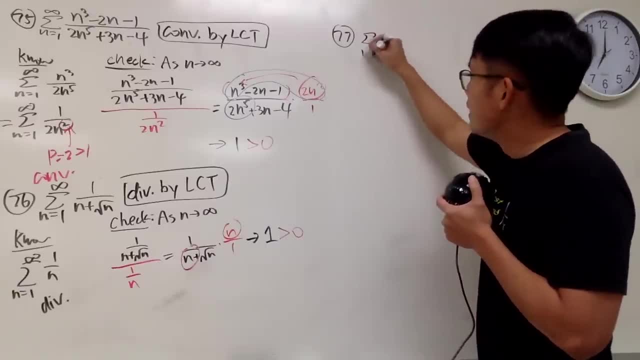 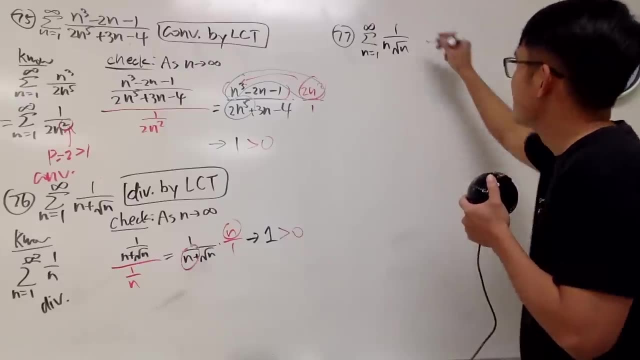 Instead of the plus sign, we have a multiplication. So here we have n equals 1 to infinity. 1 over n, square root of n. Very nice, Okay. This right here is just exactly equal to 1 to infinity. This is the same as 1 half power. 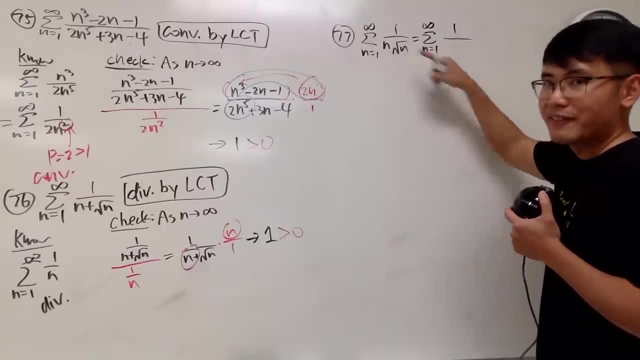 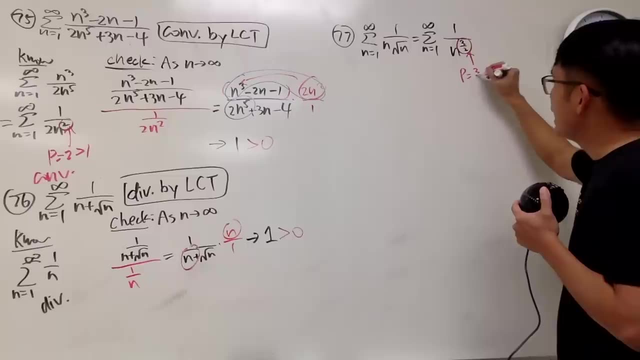 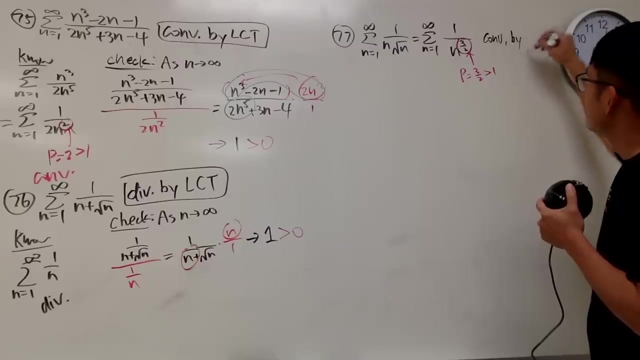 So all in all we get 1 over 1 plus 1 half. Name this 3 half power. Take a look of this right here: p is 3 half, which is greater than 1.. So this right here it converges by the p series. 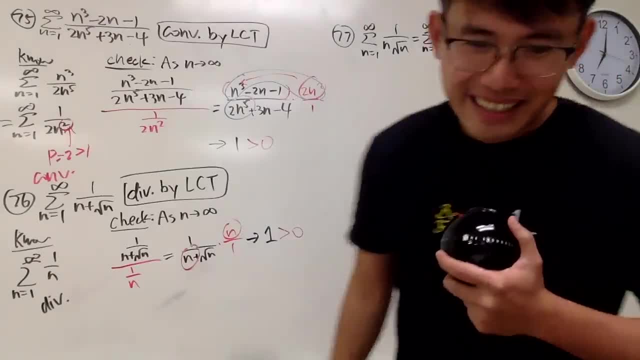 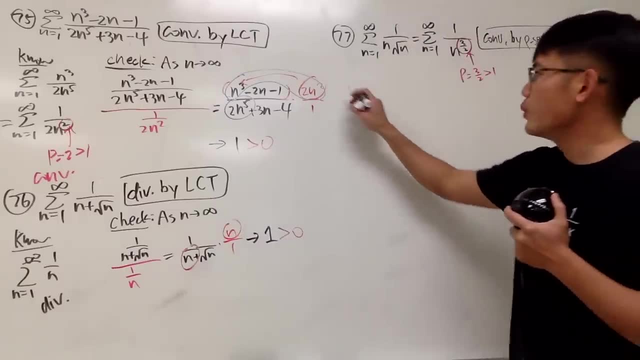 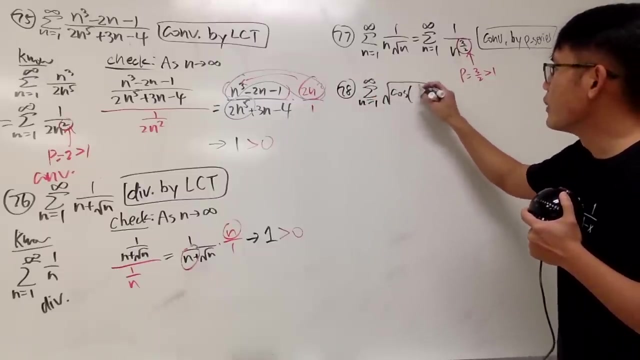 Okay, So that's it. That's it Okay. Oh, my god, square root Coming back again. huh, Trying to get us. We'll see 78, the sum as n goes from 1 to infinity. square root of cosine of 1 over n, like that. 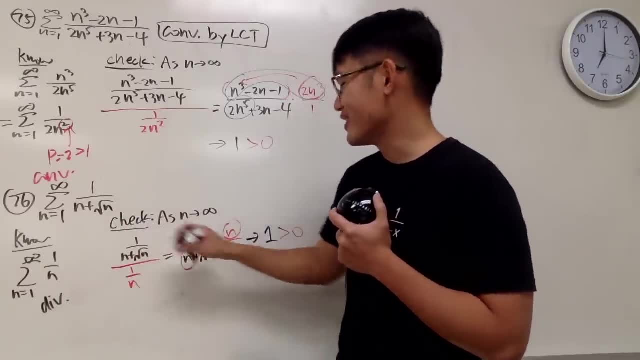 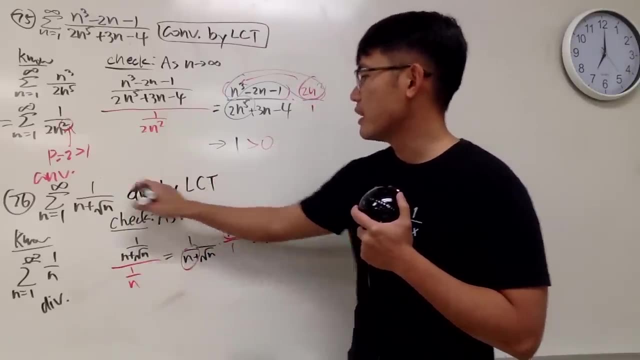 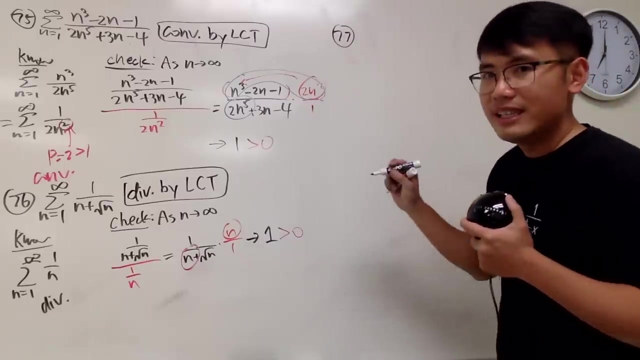 So if this diverges, this right here also diverges, because they are about the same size. This right here diverges as well by the limit comparison test, like that. Now number 77, a slightly interesting one, Not really, No, it's actually really interesting. 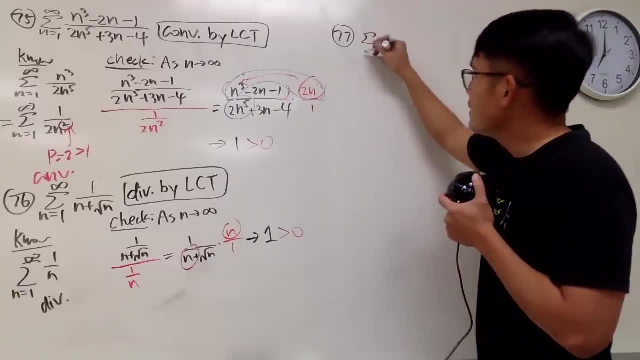 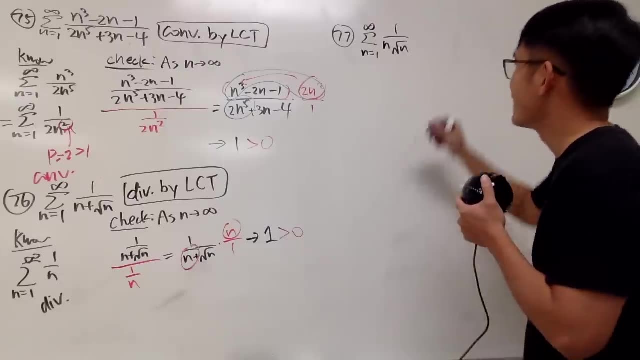 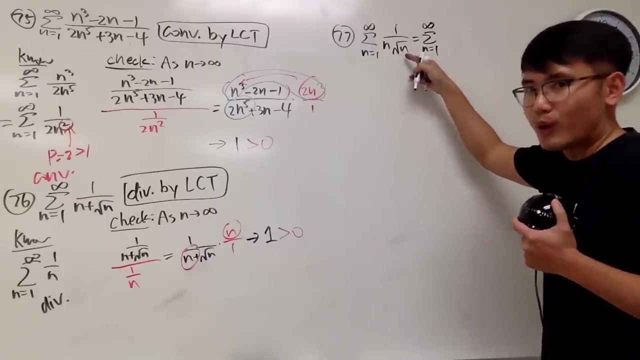 Instead of the plus sign, we have a multiplication. So here we have n equals 1 to infinity. 1 over n, square root of n. Very nice, Okay. This right here is just exactly equal to 1 to infinity. This is the same as 1 half power. so all in all we get 1 over 1 plus 1 half. 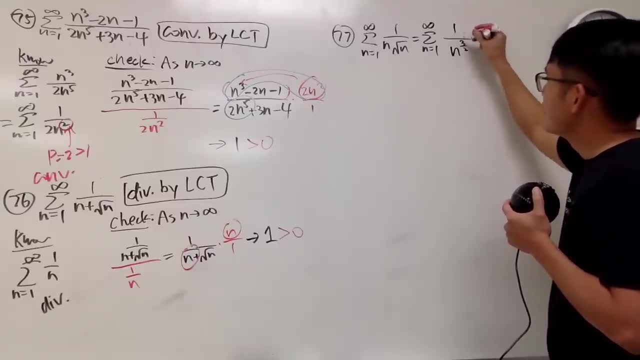 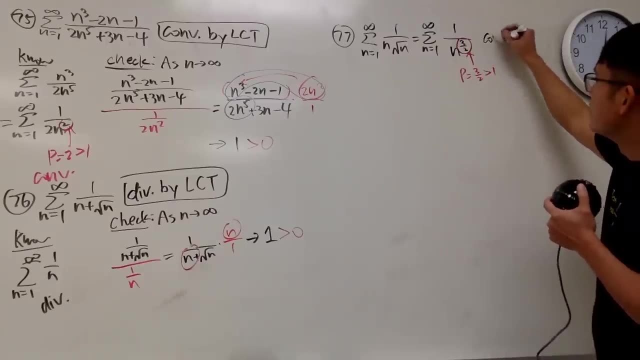 Name this 3 half power. Take a look of this right here: P is 3 half, which is greater than 1.. So this right here It converges by the p-series. Okay, So that's it, That's it. 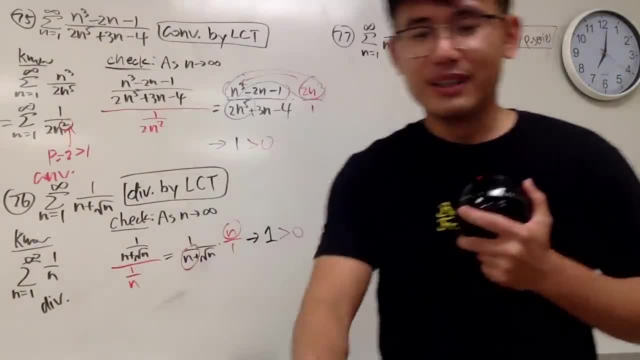 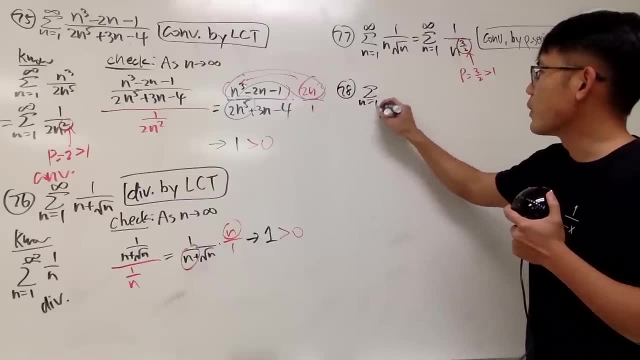 Okay, Oh, my god, square root Coming back again, huh, Trying to get us, We'll see 78, the sum as n goes from 1 to infinity. square root of cosine of 1 over n, like that. 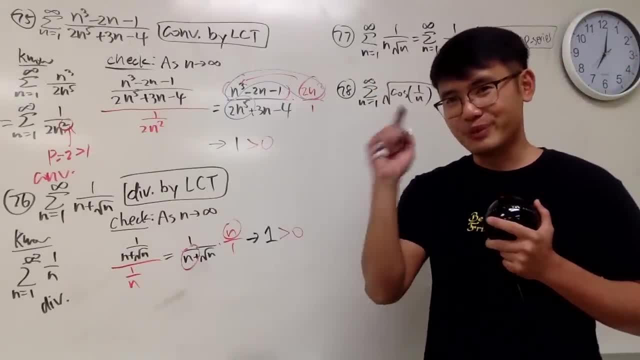 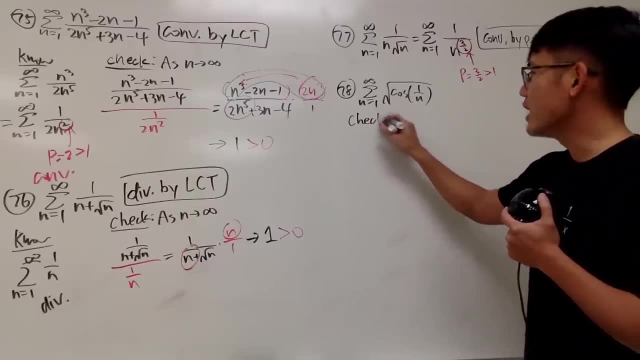 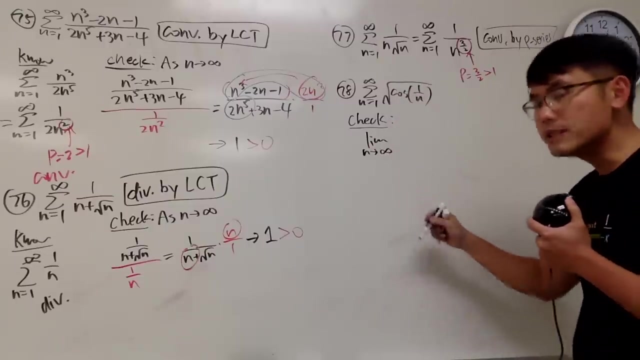 But don't forget, Cosine of 0 is 1.. This right here, it's actually just as nice, All right. So test for divergence is the way to go. Go ahead and check. Take the limit of the a, n, which is this part only, as n goes to infinity, of course. 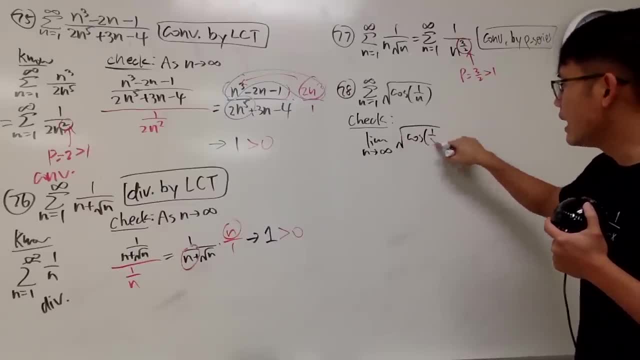 Put down the square root of cosine of 1 over n. All right, Put the infinity in here, We get just like 1 over infinity, which is 0. And all in all, you just get 1.. Seriously, Cosine of. let me just show you guys a little bit more work. 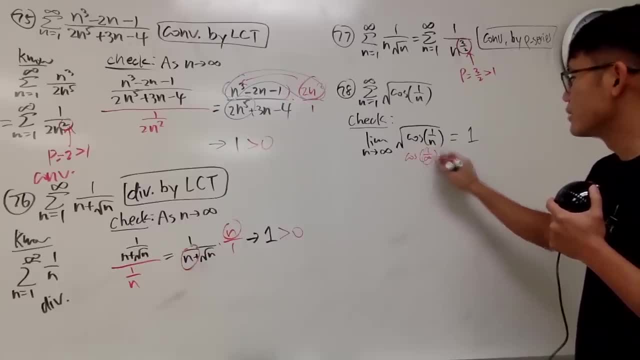 Cosine of 1 over infinity, which is this right here, is just 0.. Cosine of 0 is 1.. Square root of square root of 0, no, square root of 1 is still 1.. So this right here. divergence by test for divergence: t, f, d right. 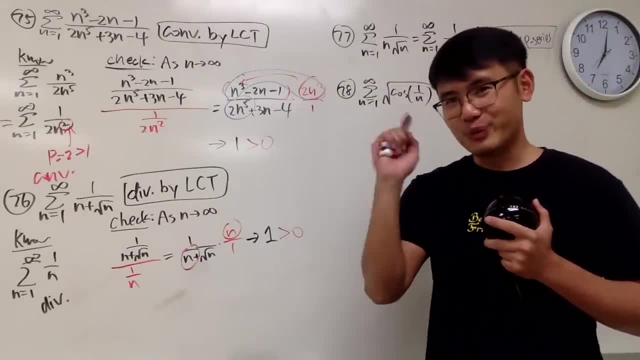 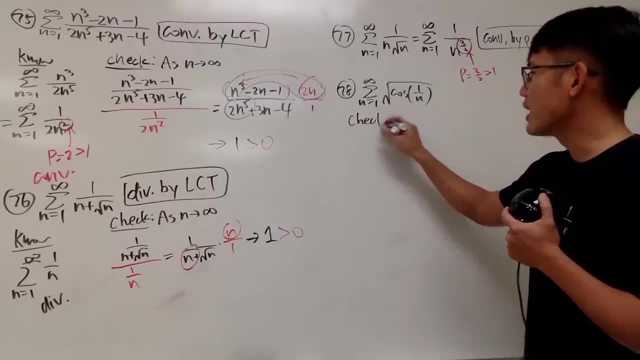 But don't forget, cosine of 0 is 1.. This right here, it's actually just as nice, All right. so test for divergence is the way to go. Go ahead and check. Take the limit of the a- n, which is this part only. 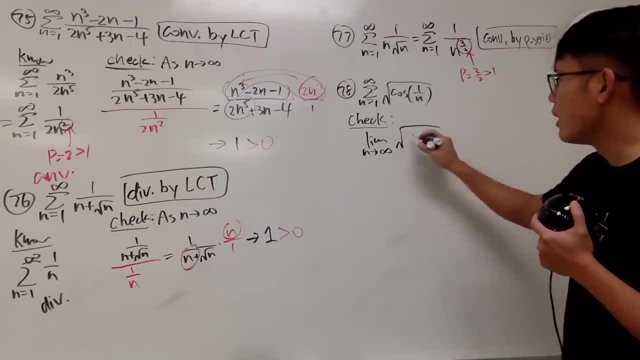 as n goes to infinity. of course, Put down the square root of cosine of 1 over n. All right, Put the infinity in here, We get just like 1 over infinity, which is 0. And all in all you just get 1.. 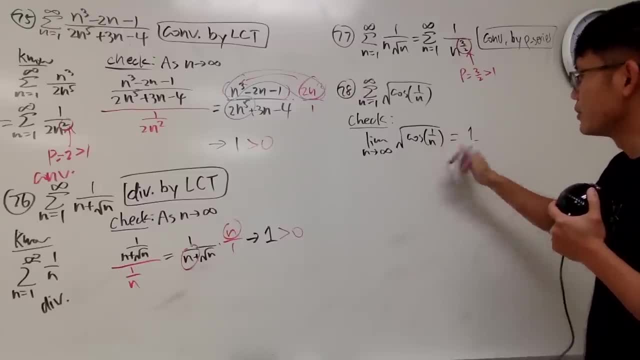 Seriously, cosine of. Let me just show you guys a little bit more work. Cosine of 1 over infinity, which is This right, here is just 0.. Cosine of 0 is 1.. Square root of 0.. 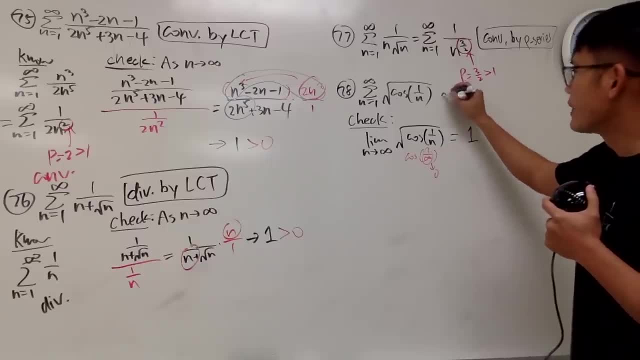 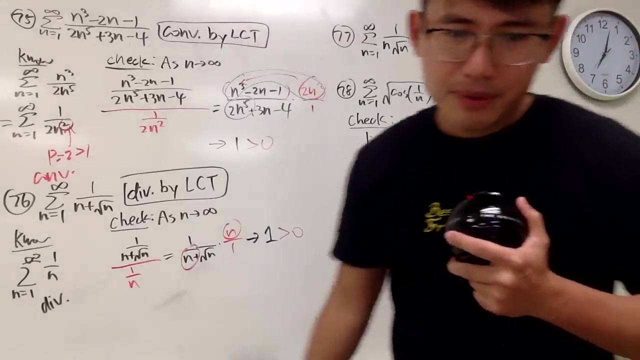 Square root of 1 is still 1.. So this right here. divergence by test for divergence: T, F, D, right. So it looks scary, but it's actually not that bad at all. Now number 79.. Oh, I remember this. 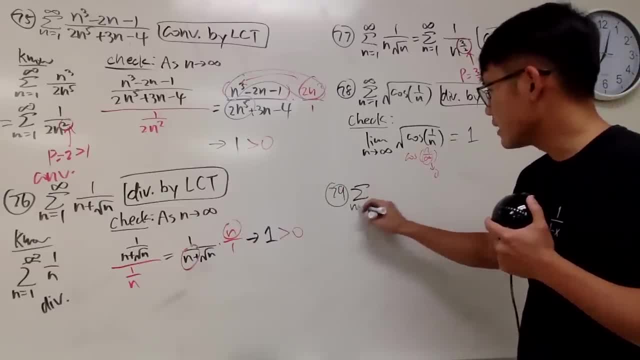 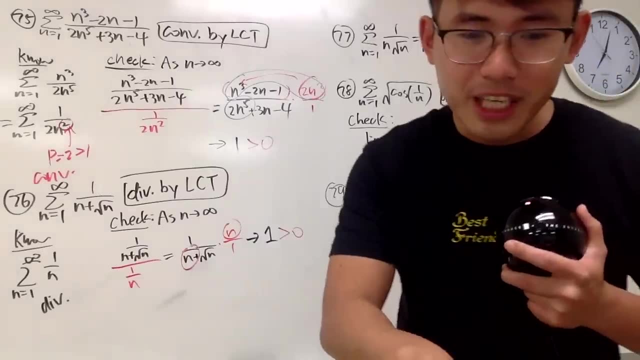 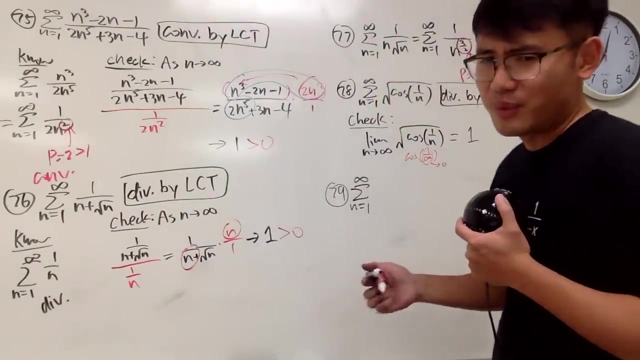 One of the ones you'll see a lot. The sum as n goes from 1 to infinity- Infinity. Here We are going to team up the exponential and then the power function with, Then try to beat with the factorial. We'll see if it works or not. 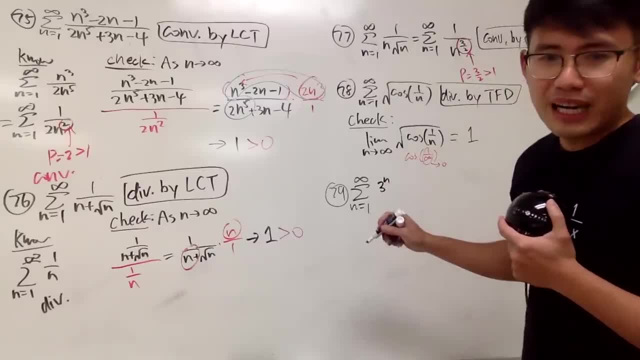 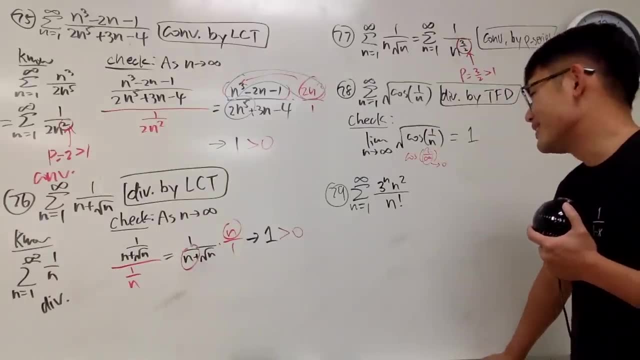 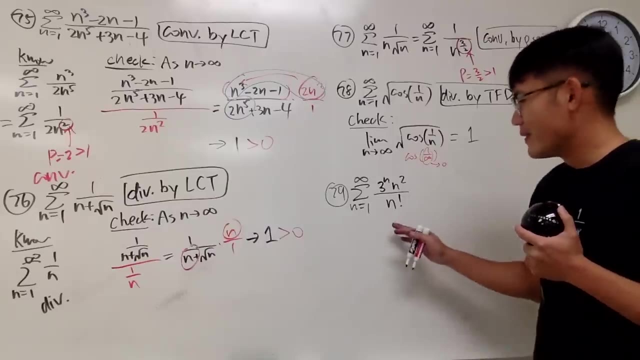 I don't know. 3 to the n And we have n squared over n- factorial. Hmm, In fact we did this kind of thing earlier, but let's just try this again. Do you guys think convergence diverges Okay? 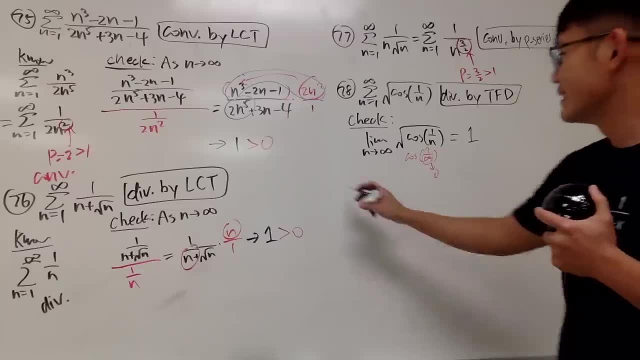 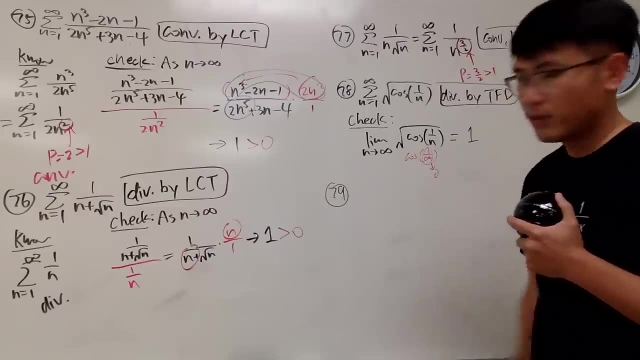 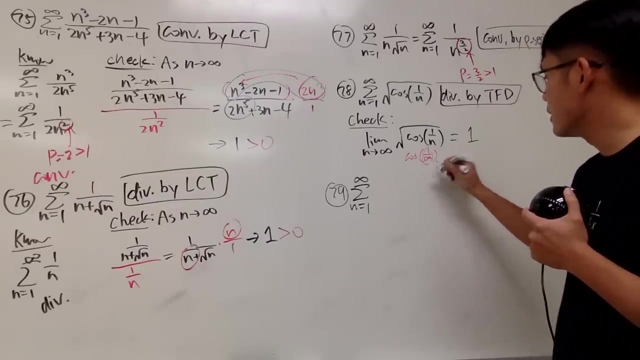 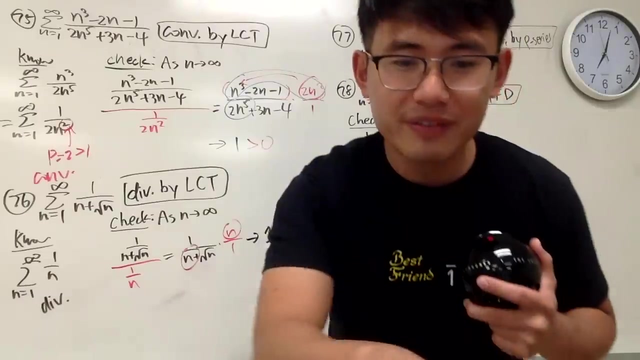 So it looks scary, but it's actually not that bad at all. Now Number 79.. Oh, I remember this, One of the one. you'll see a lot. The sum as n goes from 1 to infinity. Here we are going to team up the exponential and then the power function with. 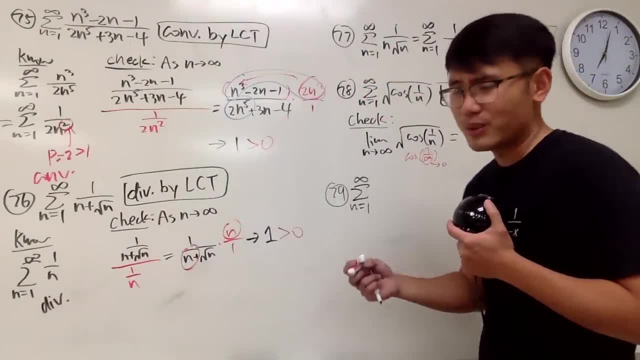 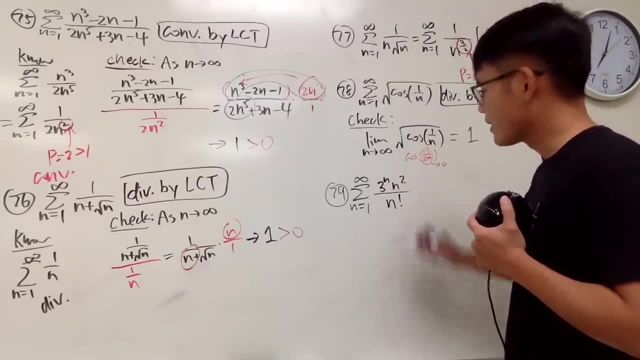 then try to beat with the factorial. We'll see if it works or not, I don't know. 3 to the n, And we have n squared Here over n factorial. Hmm, In fact we did this kind of thing earlier, but let's just try this again. 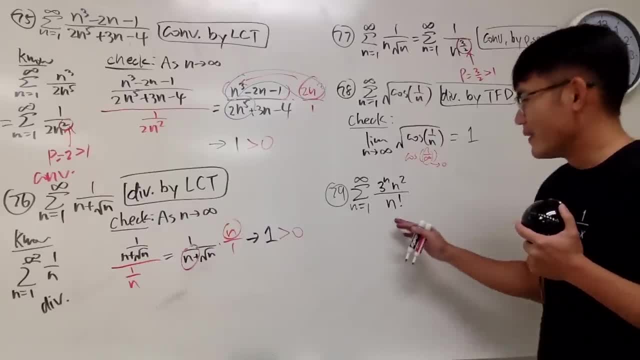 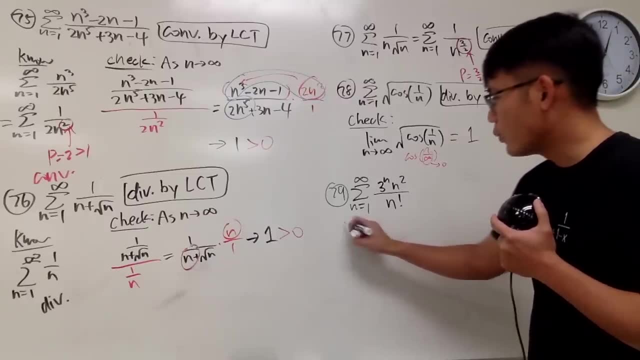 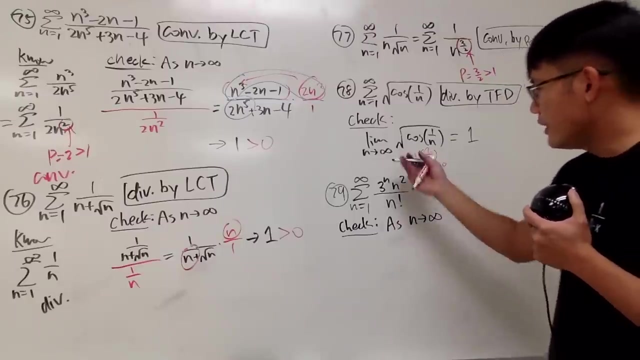 Do you guys think convergence diverge? Okay, Let's see, Right here, of course, let's go ahead and use the ratio test. So we are going to check right As n goes to infinity. This right here. we take the absolute value of 3 to the n plus. 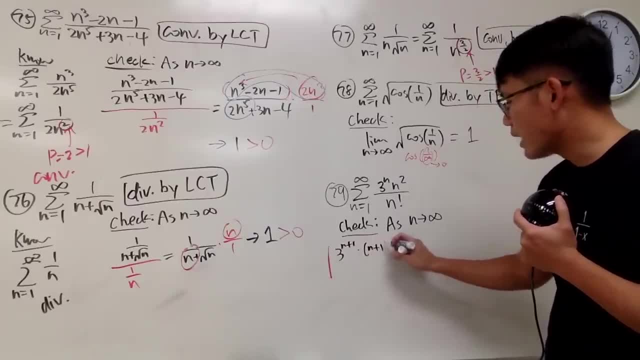 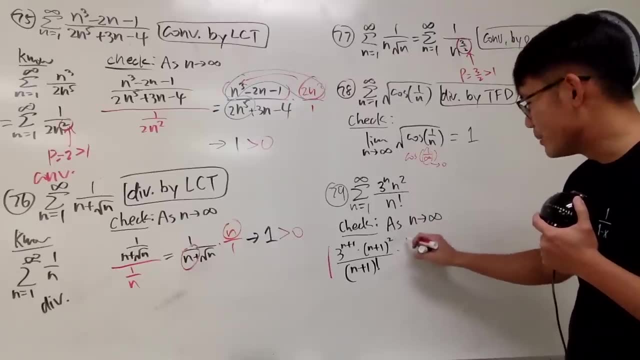 plus 1 power times n plus 1 squared over n plus 1, parentheses. and you do the factorial and then you put the reciprocal here n factorial over 3 to the n times n, squared like this: 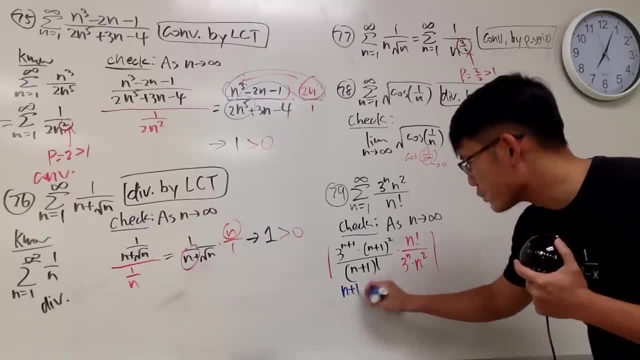 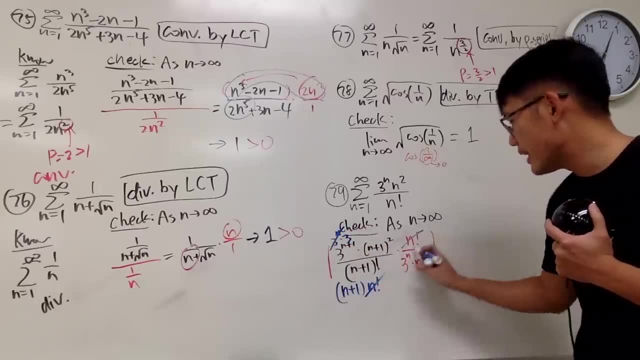 Now here is the deal Again: this: right here: n plus 1, times n factorial: this and that. cancel This. right here, 3 to the n times 3, this and that cancel. So so far we are actually: let's cancel this and that again. 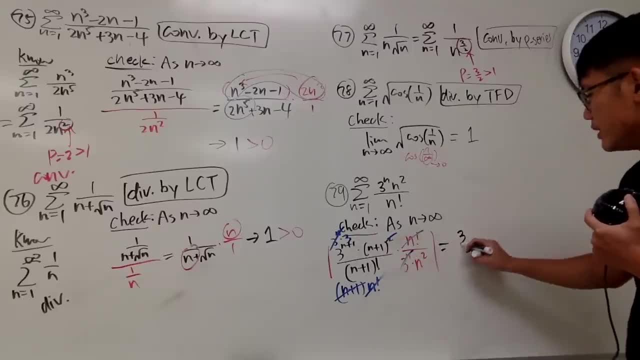 So you see, on the top this is just 3, parentheses n plus 1, and over n, squared like that, Similar to the one we did earlier, It approaches 0.. And this is the ratio test. Remember when the ratio test gives you 0 right here, this is actually good. 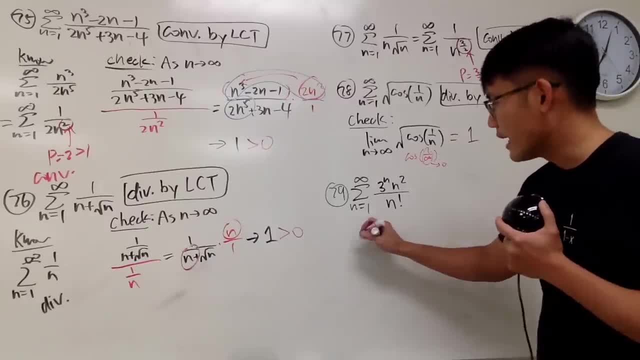 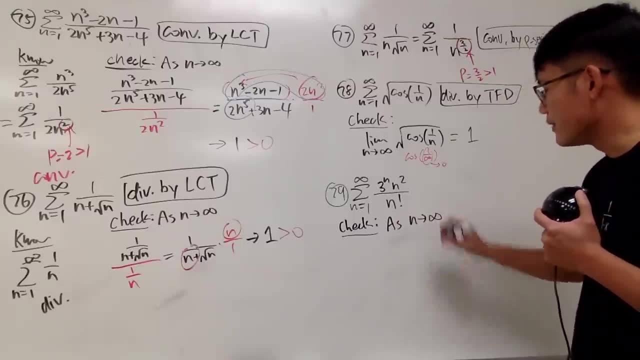 Let's see Right here, of course, let's go ahead and use the ratio test. So we are going to check. Okay, As n goes to infinity, This right here. we take the absolute value of 3 to the n plus 1 power. 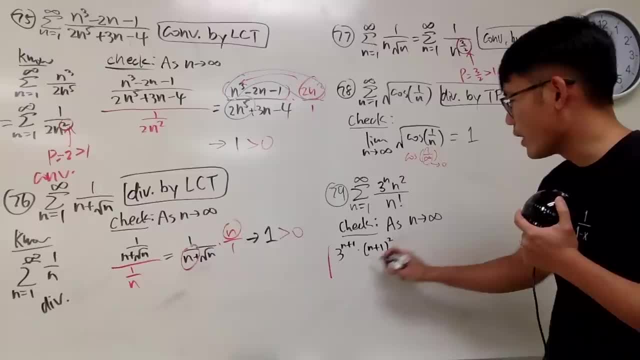 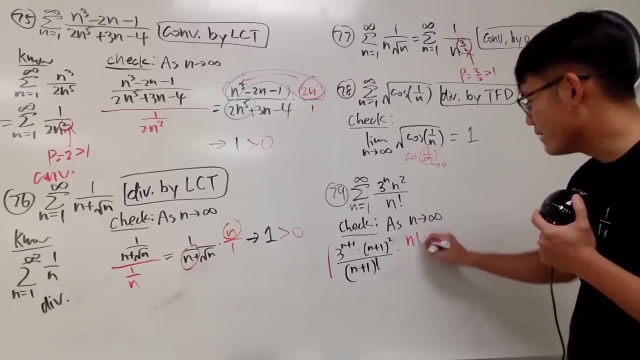 times n plus 1 squared over n plus 1.. Parenthesis is C and you do the factorial And then you put the reciprocal, here n factorial over 3 to the n times n, squared, like this. Now, here is the deal. 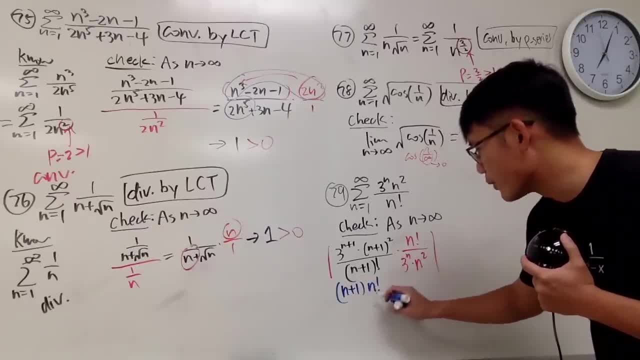 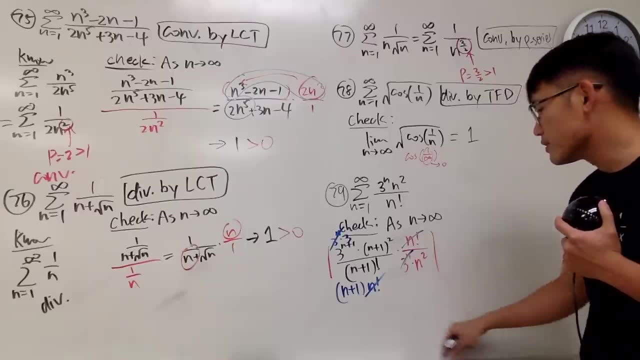 Again this right here: n plus 1 times n factorial. This and that. cancel This right here: 3 to the n times 3.. This and that cancel. So so far we are actually, Let's cancel this and that again. 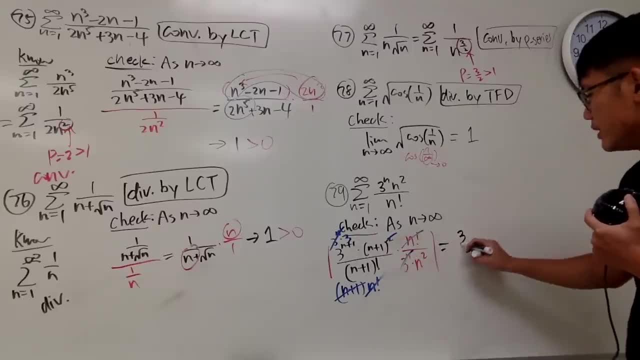 So you see, on the top this is just 3 parenthesis n plus 1. And over n, squared like that, Similar to the one we did earlier, It approaches 0.. And this is the ratio test. Remember when the ratio test gives you 0 right here, this is actually good. 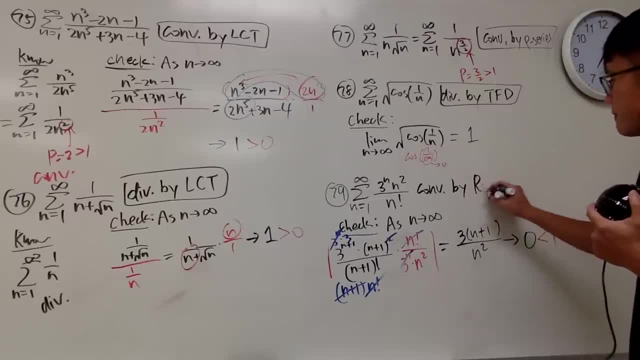 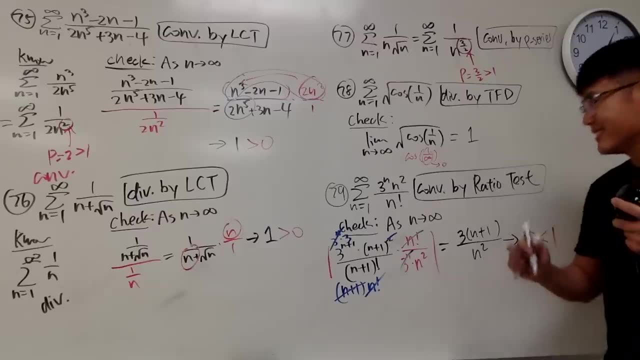 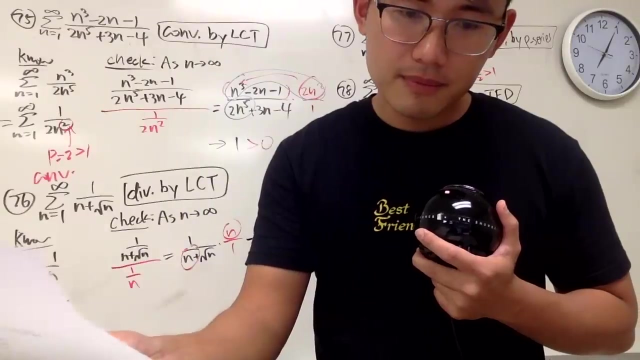 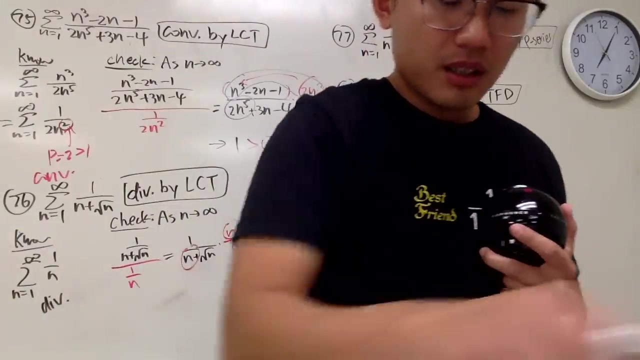 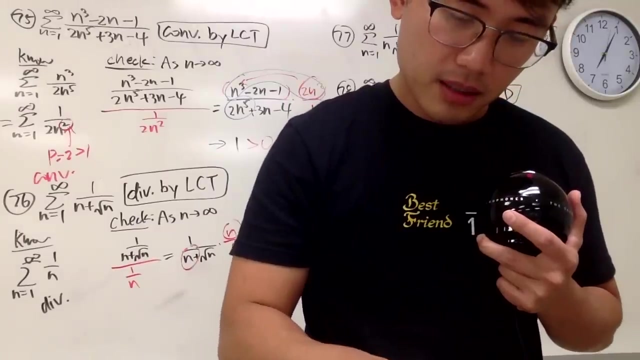 This right here converges by the ratio test, Right? So that's very nice, Right? Hmm, Okay, Okay, Okay, Okay, Okay Okay, Of course I will make some mistake. Take number 90.. Take a look. 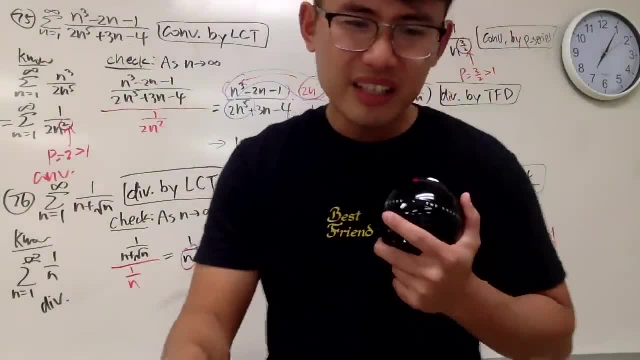 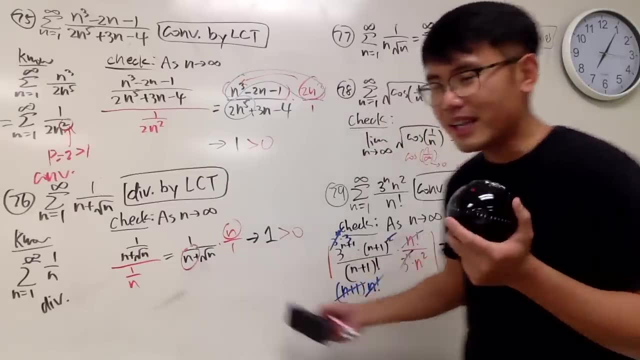 If you look at number- Sorry, number 80, we have the n and then the 2n. In fact we did that in question number 30 already. right, But no, Yes, But yes. Well, yes, I mean yes. 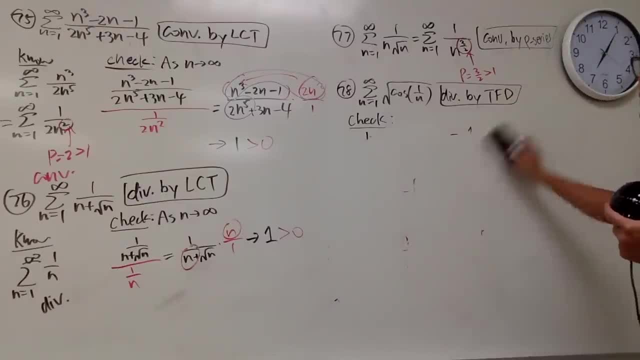 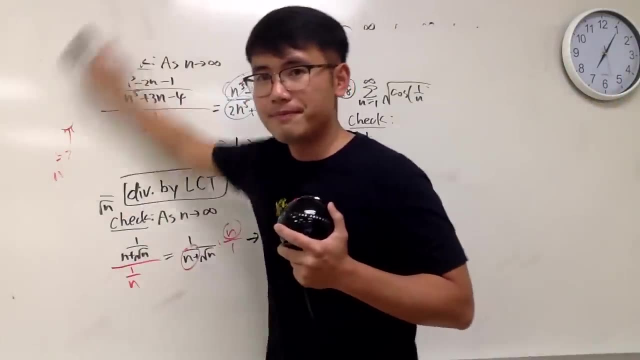 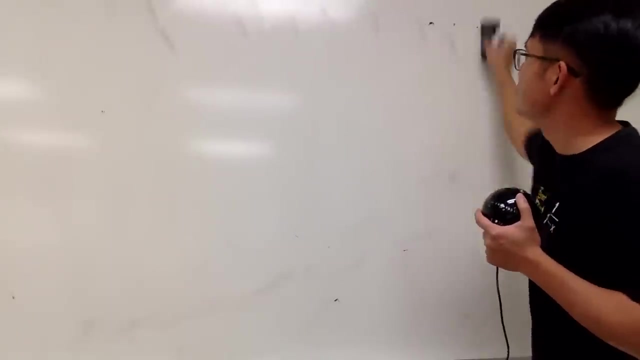 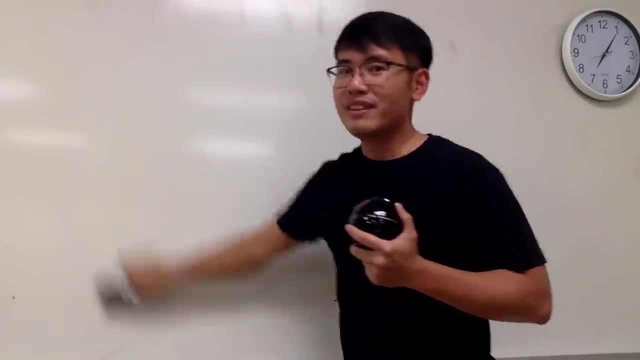 But no, don't worry, I will show you guys another way to do this. Okay, Okay, so we're gonna see how to work this out. number 80: oh my god. 20 more questions to go. this is like mile like 20, uh, for my mirror zones and, to be honest, today i forgot my mirror zone. 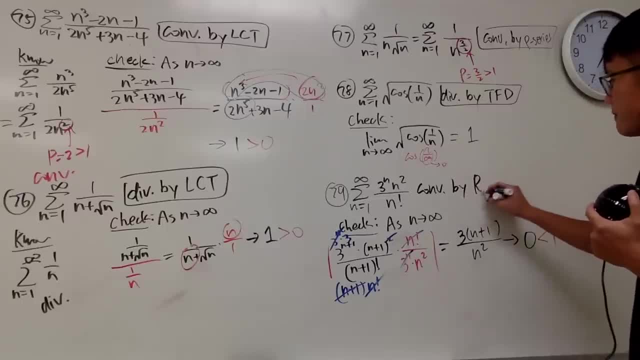 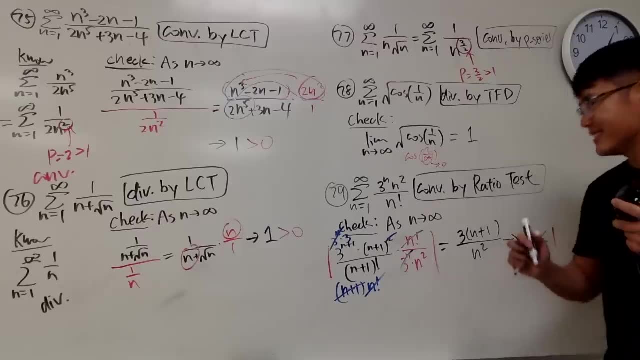 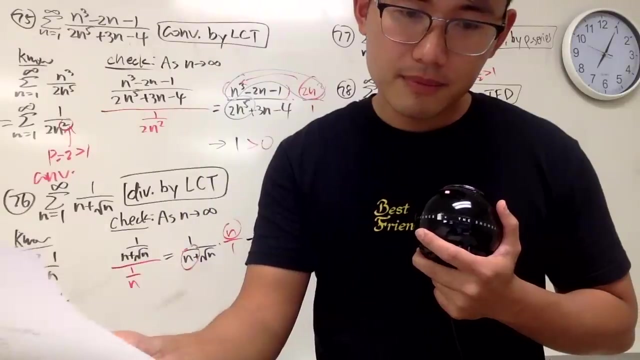 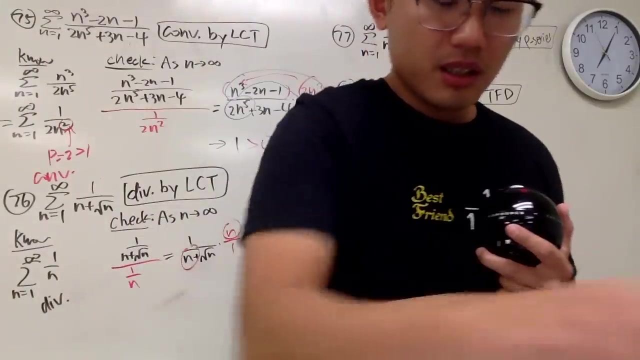 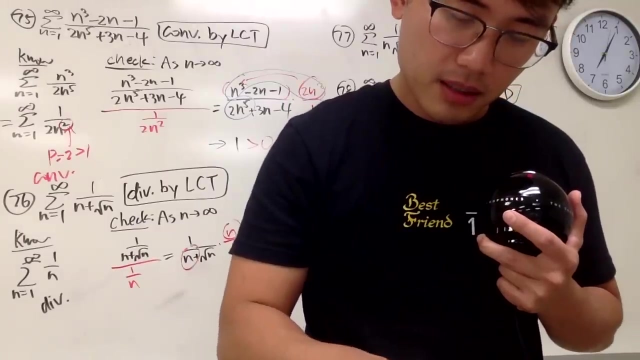 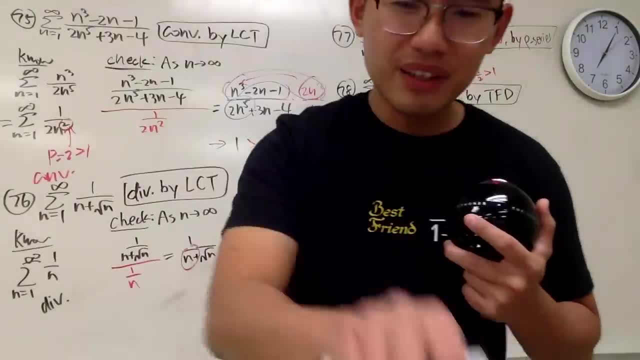 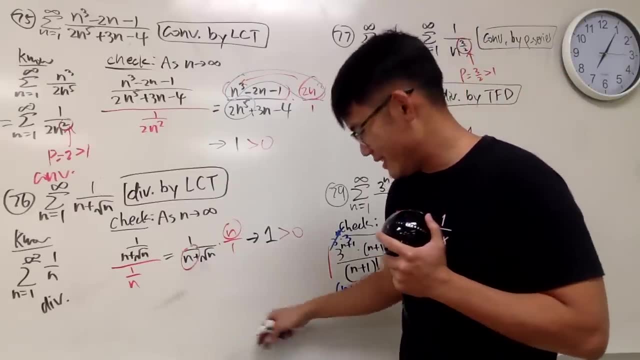 90.. 90., 90. Look, if you look at number- sorry, number 80, we have the n and then the 2n. In fact we did that in question number 30 already. right, But no, yes, but yes, well, yes, I mean yes. 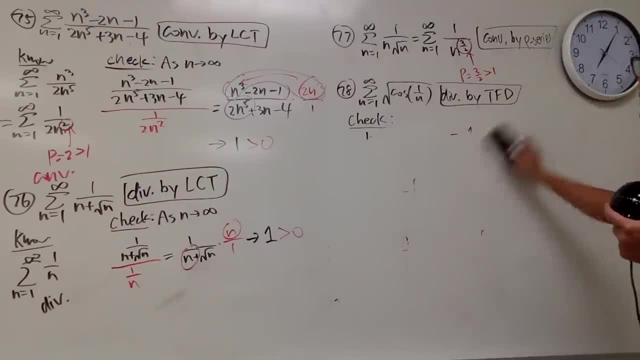 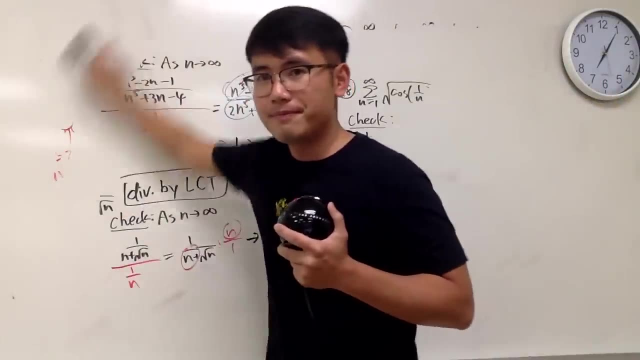 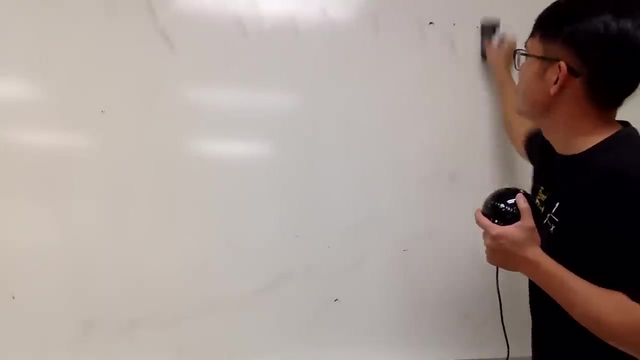 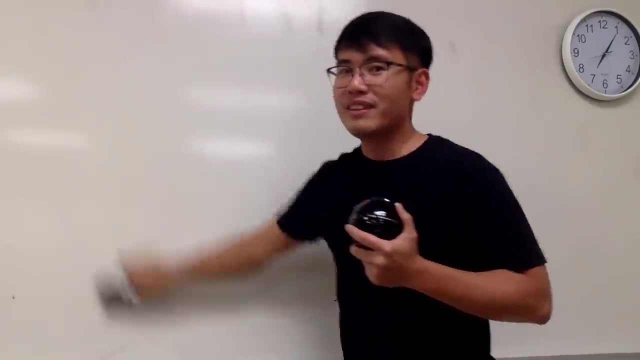 But no, don't worry, I'll show you guys another way to do this. So we're going to see how to work this out. number 80.. Oh my god, 20 more questions to go. This is like my old, like 20 for my mirror zones. 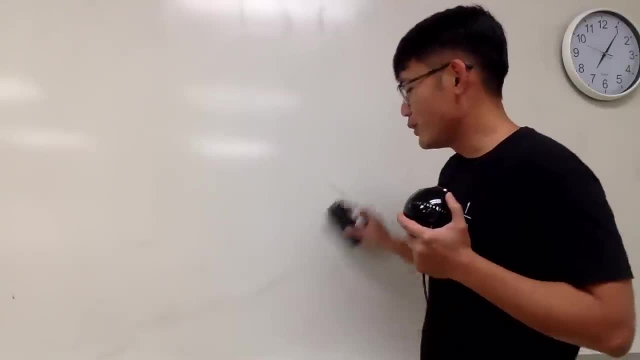 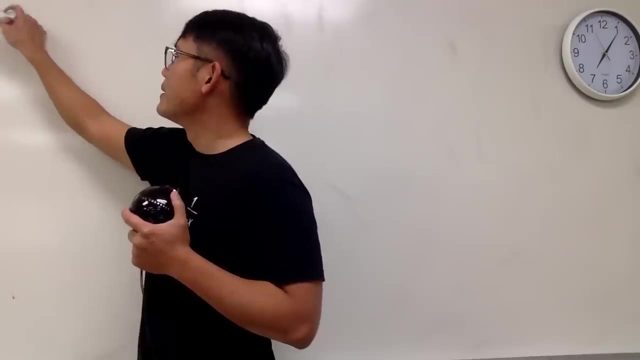 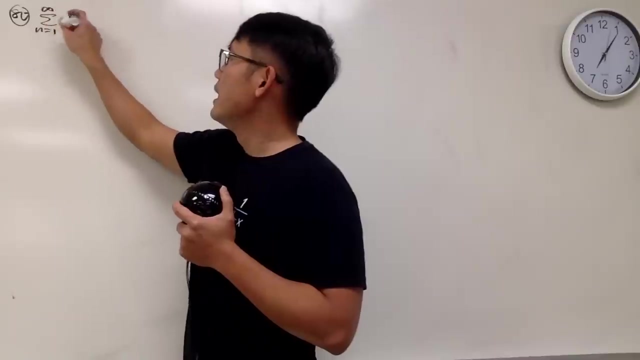 And, to be honest, today I forgot my mirror zone medal. Otherwise, I really want to put a mirror zone medal after I finish doing all this, but maybe next time. Anyway, number 80 right here. This time we are going to find the sum as n goes from 1 to infinity, n over 2 to the n. 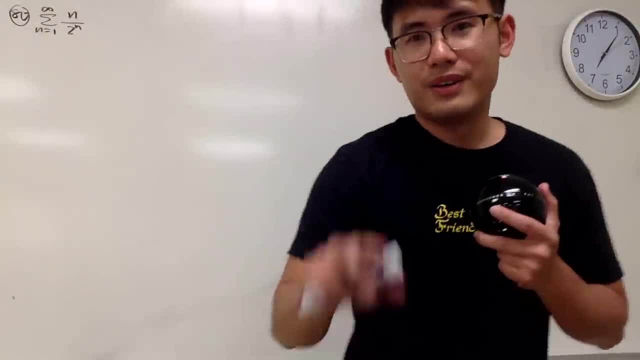 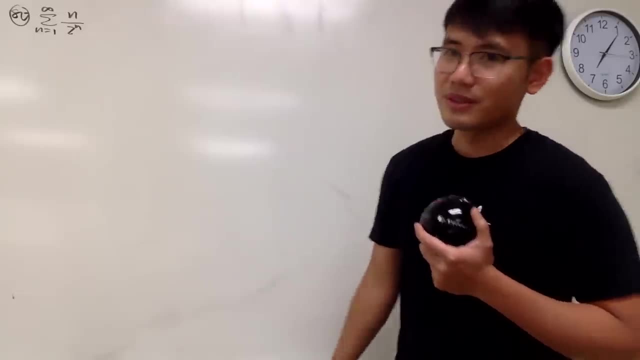 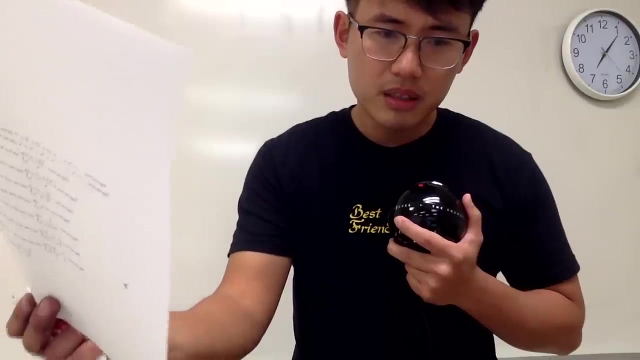 And if you guys look at these questions, power series- okay, A lot of power series will be coming. so that's the idea. So here is the deal. let's see, Yeah, let's do that- Power series in action. 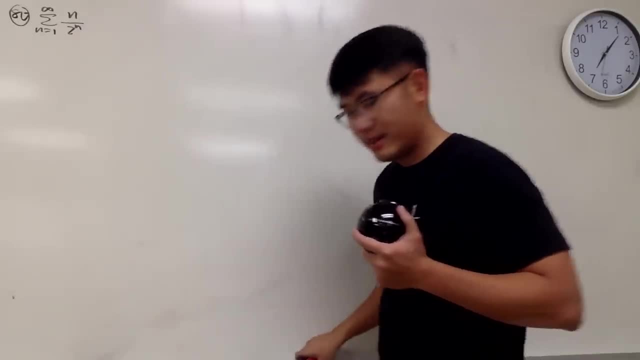 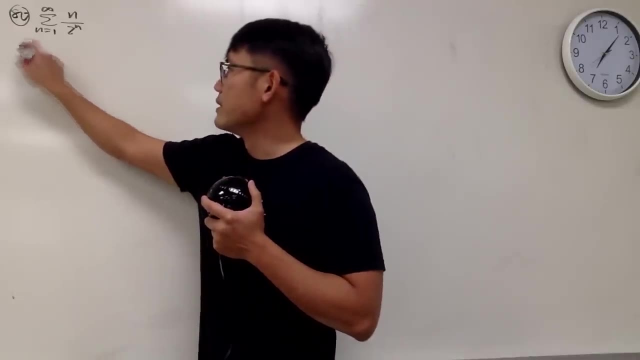 I'm not going to use the meta idea earlier, so now let's recall best friend To help us out. So this is the work that we are going to do, So recall our best friend, right? So this is the best friend. 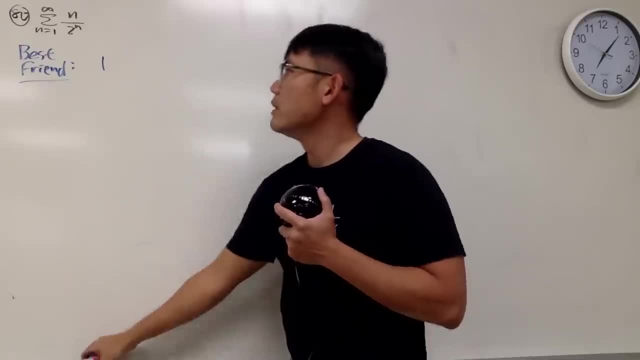 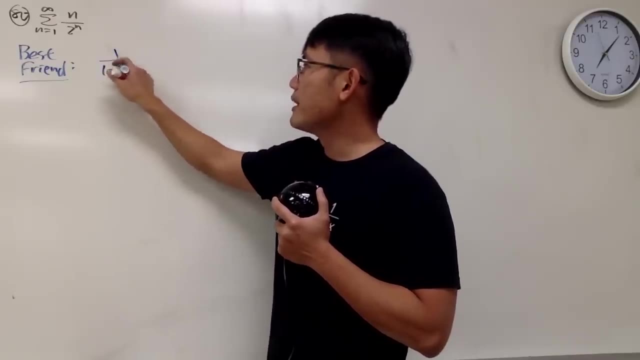 First, we know that 1, I'll just write it down like this: We know that if we have 1 over 1 minus x, this right here, thanks to the best friend, we know this is the sum as n goes from 0 to infinity. 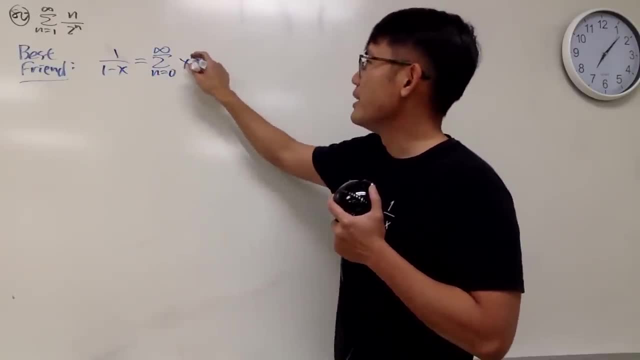 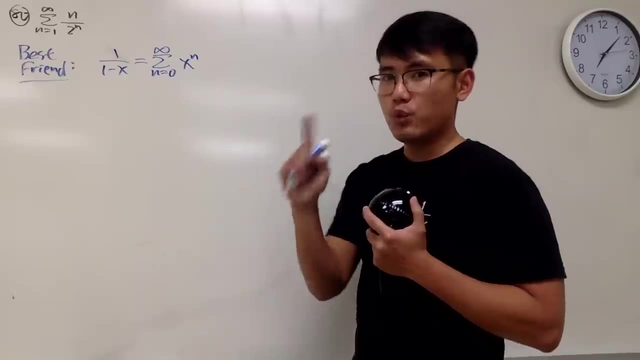 This is going from 0 to infinity. And then here we have x to the nth power. By the way, in power series we will have a convention that 0 to 0 is 1.. It's just a convention when we have the sigma notation and all that in power series, right? 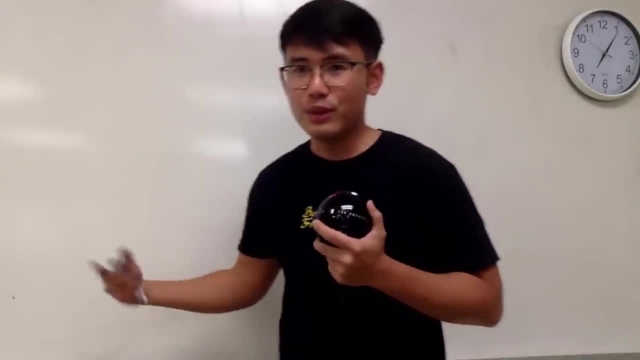 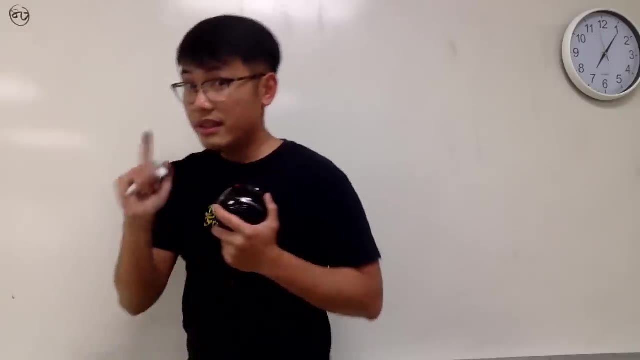 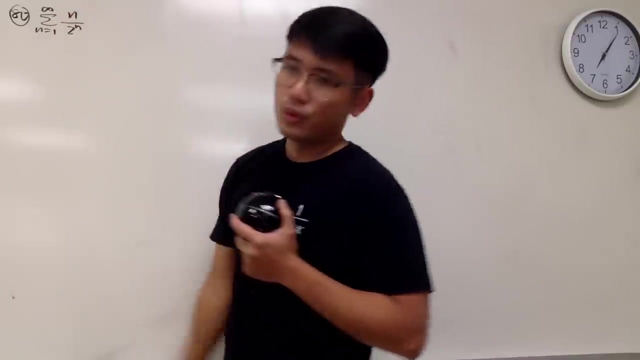 medal. otherwise i really want to put a measure of metal after i finish doing all this, but, um, maybe next time. anyway, number 80 right here. this time we are going to find the sum as n goes from 1 to infinity and over 2 to the n. and if you guys look at these questions, 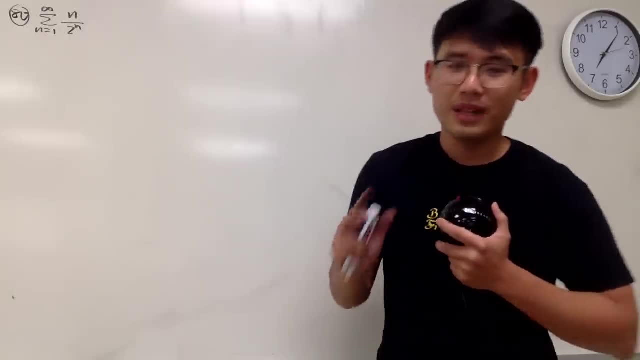 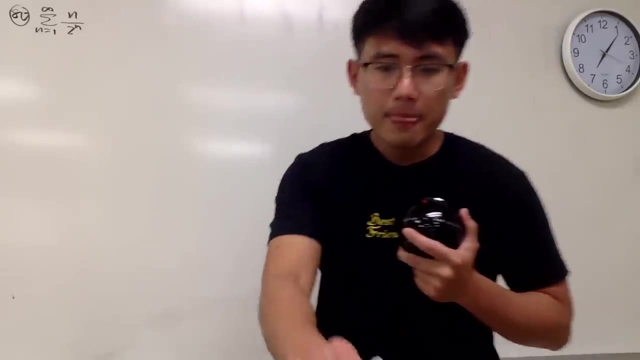 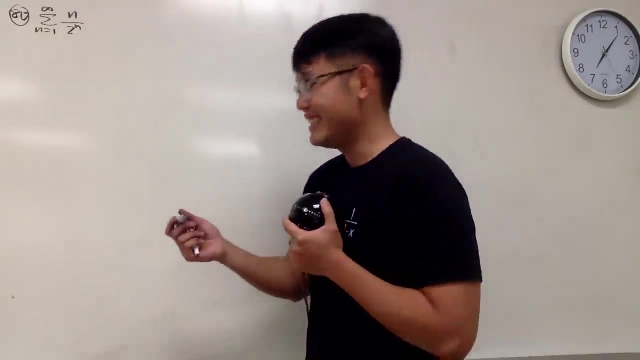 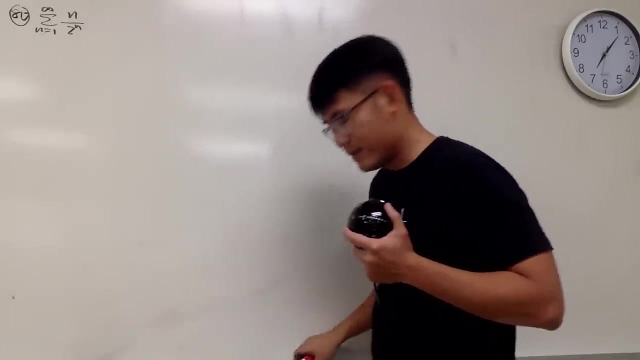 power series. okay, a lot of power singers. power series will uh, coming and will be coming. so that's the idea. so here is the deal. let's see, yeah, let's do that- power series in action. i'm not going to use the meta idea earlier, so now let's recall best friend to help us out. 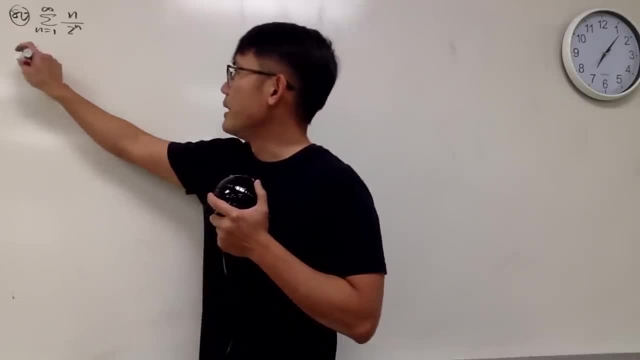 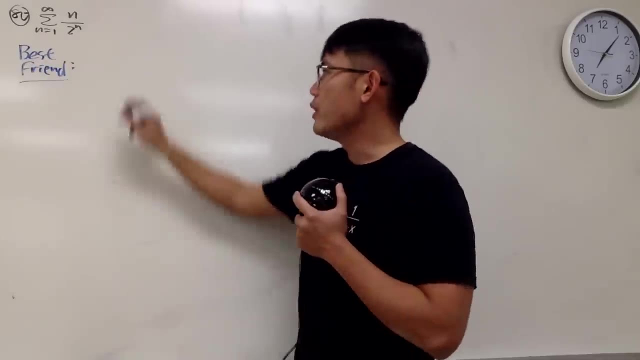 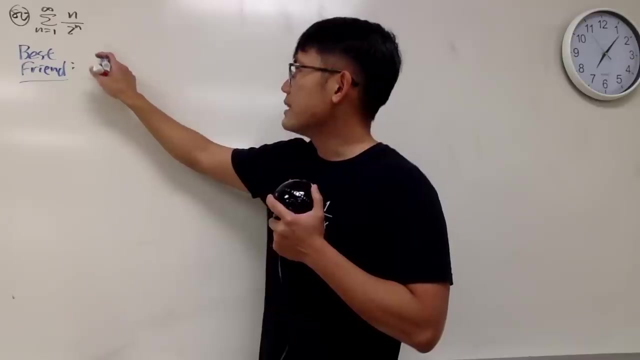 so this is the work that we are going to do. so recall our best friend. so this is the best friend. first. we know that one. i'll just i'll just write it down like this: we know that if we have 1 over 1 minus x. 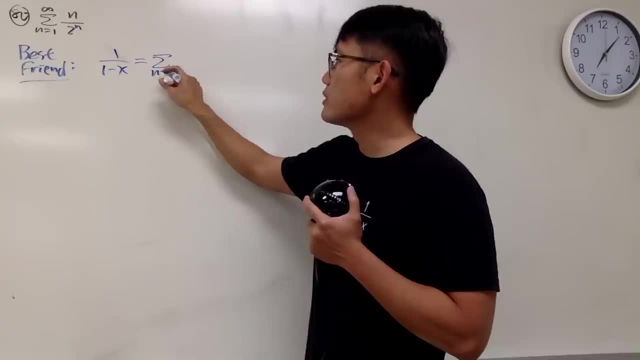 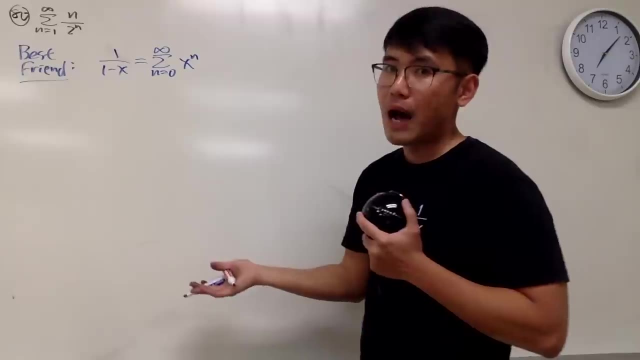 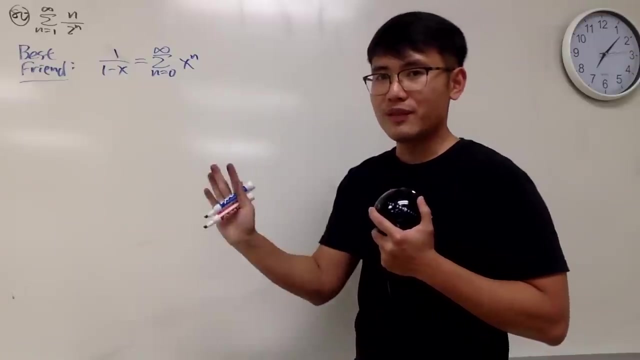 this right here, thanks to the best friend. we know this is the sum, as n goes from 0 to infinity. this is going from 0 to infinity, and then here we have x to the nth power. by the way, in power series we will have a convention that 0 to 0 is 1. it's just a convention where we have the sigma notation and 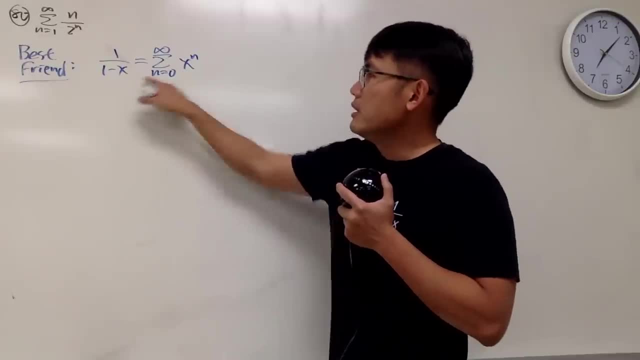 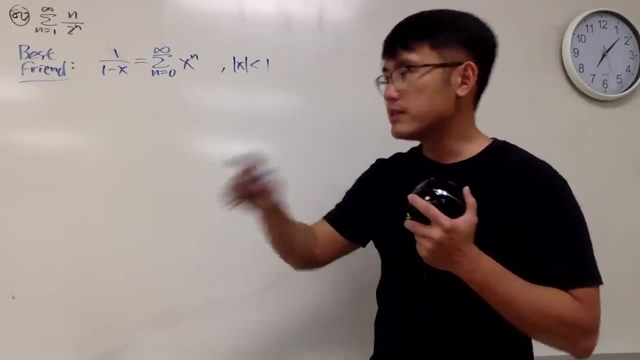 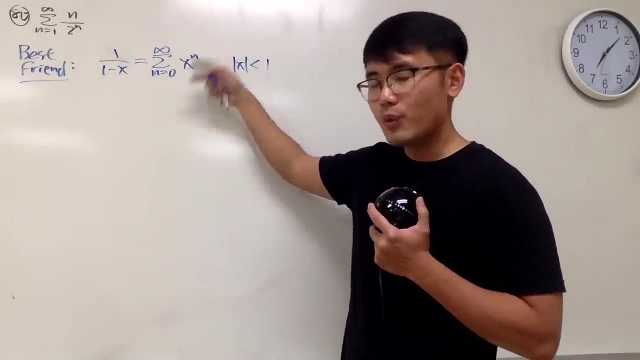 the power series right, because you can imagine, this is true when the absolute value is less than 1, so it should be true when x is 0 as well, and if you're putting 0 on the left hand side, you have 1. on the right hand side you have 0 to the nth power, and since n goes from 0, 1 to 3, and so on. 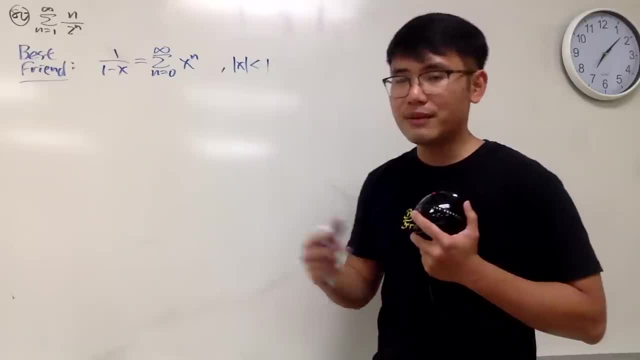 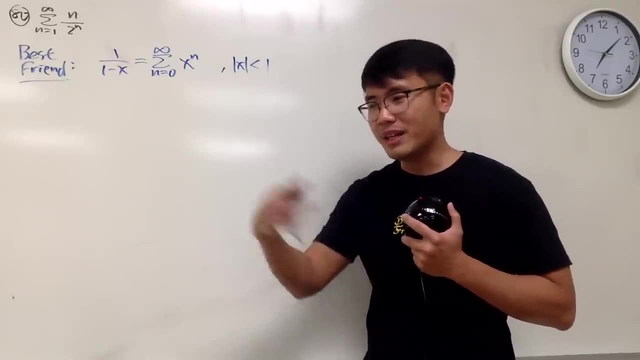 the first time is 0 to the 0th power. so you really have to just take a convention that 0 to 0 is 1 in the power series situation. i'm not saying 0 to 0 is always equal to 1 in the other. 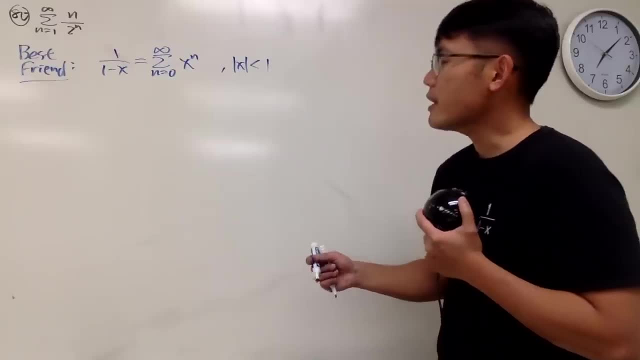 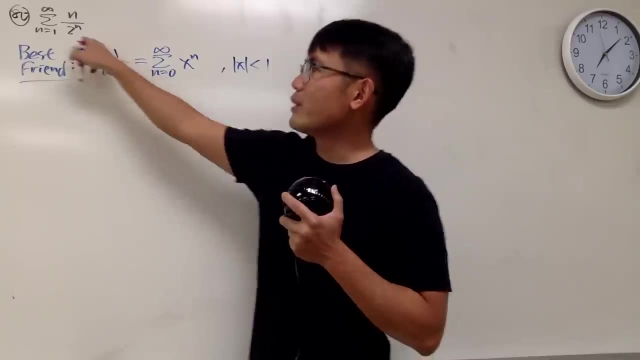 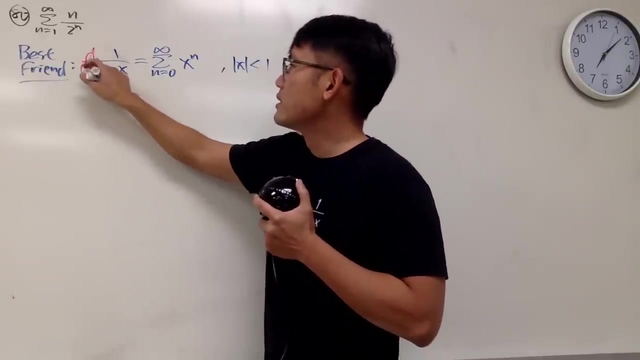 context. but yeah, in this case, yeah, all right. so this is how we're going to do it. we are going to do the derivative. so, because you can see that if you put one half, you get 2 to the n right one half here. so that's a geometric. you have this n, so we do the derivative on both sides. so here we go. 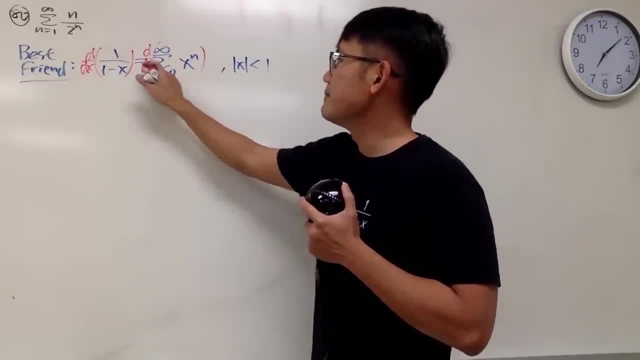 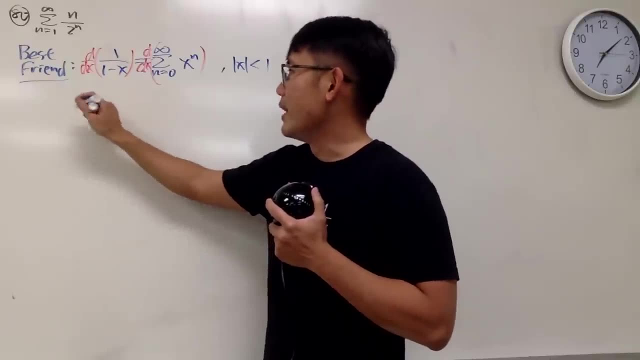 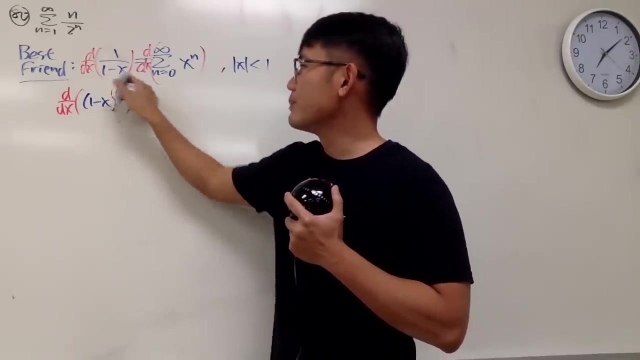 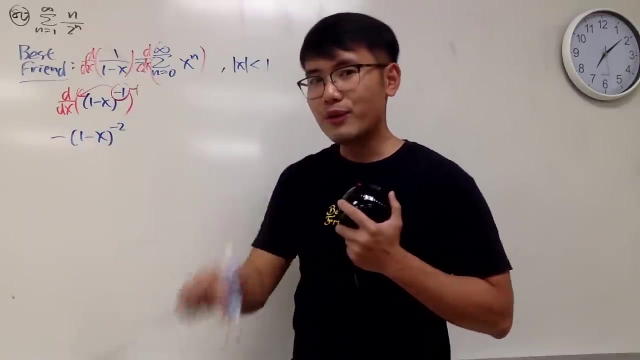 differentiate this and differentiate that on the 11th side. okay, you can do it this way: differentiate 1 minus x to the negative 1 power. of course, bring this to the front minus 1, so we get negative parentheses. 1 minus x to the negative 2 power. but don't forget the chain loop. multiply by. 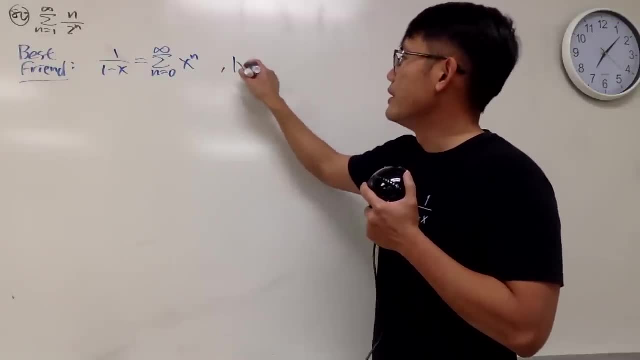 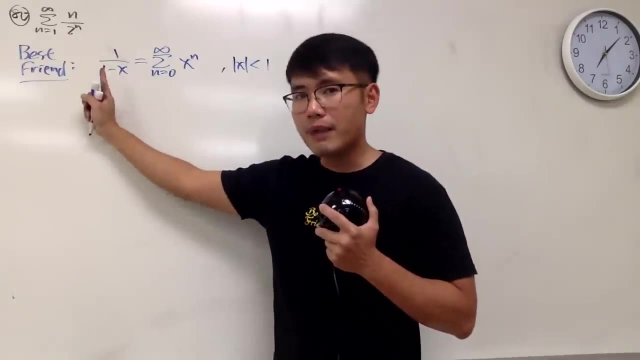 Because you can imagine, this is true when the absolute value is less than 1.. So it should be true when x is 0 as well. And if you're putting 0, on the left-hand side, you have 1, on the right hand side, you have 0 to nth power. 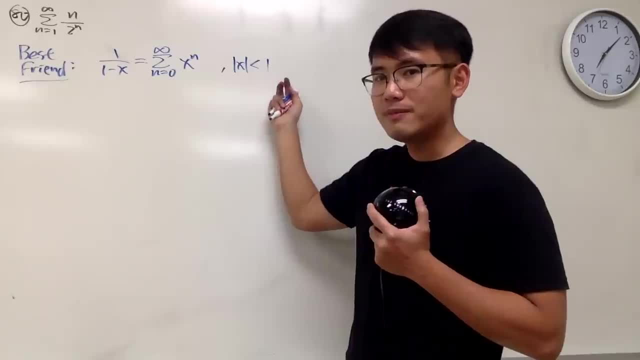 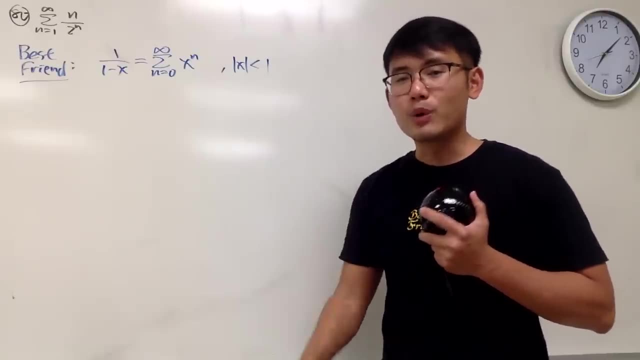 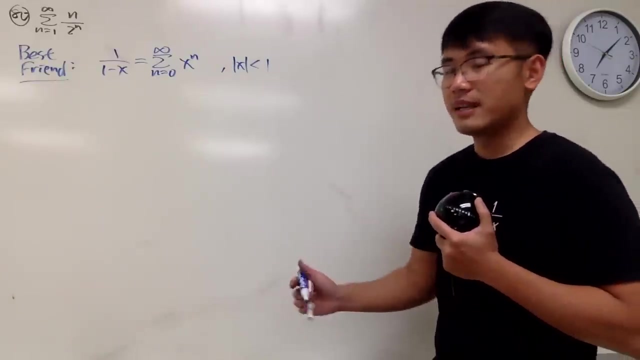 and since n goes from 0, one, two, three and so on, the first time is zero to the zeros power. so you really have to just take a convention that zero to a zero is one in the power series situation. i'm not saying zero to zero is always equal to one in the other context, but yeah, in this case. yeah, all right. so this is. 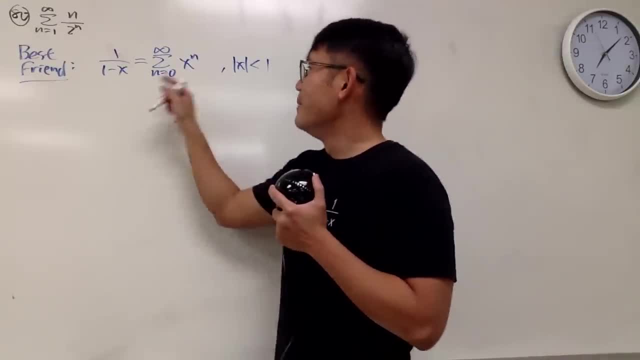 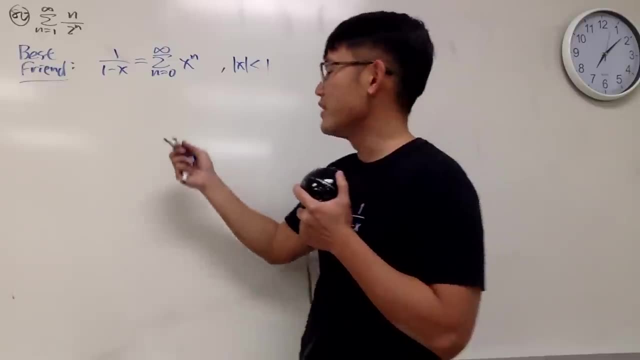 how we're gonna do it. we are going to do the derivative. so, because you can see that if you put one half, you get two to the end, right, one half here. so that's a geometric. you have this, and so we do the derivative on both sides. so here we go, differentiate this and differentiate that. 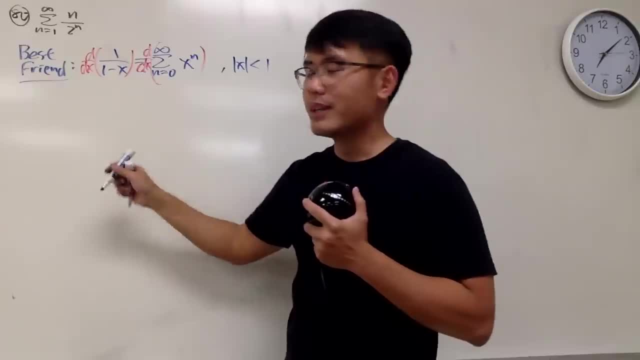 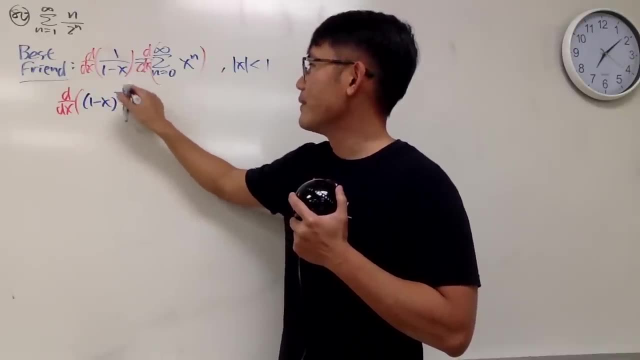 on the 11 side. okay, you can do it this way: differentiate 1 minus x to the negative 1 power, of course, bring this to the front minus 1, so we get negative parentheses. 1 minus x to the negative 2 power. but don't forget the chain loop. 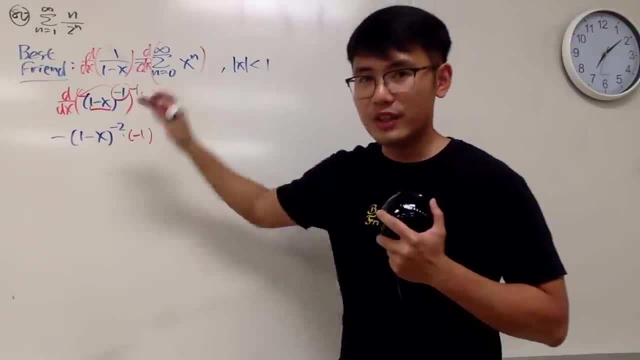 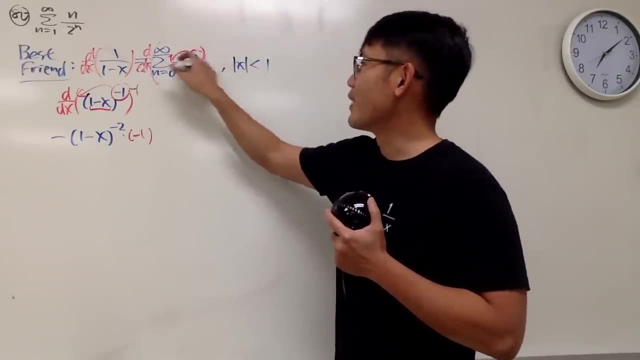 we're going to you, multiplied by the derivative inside, which is multiplied by negative 1, like this We differentiate this right here. On the left-hand side, you just differentiate x to the nth power. bring this to the front minus 1.. 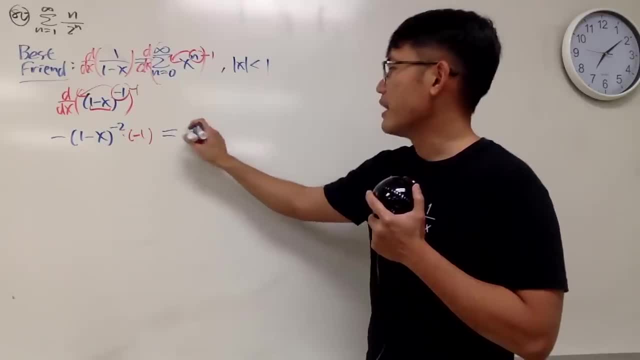 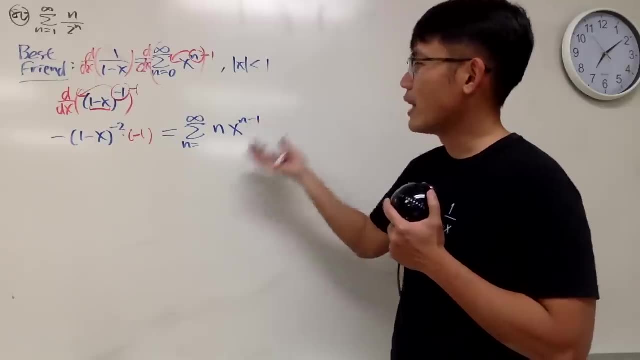 So let me write this down right here for you guys. This is actually the same as saying the sum, as n goes from something to infinity and you have n x to the n minus 1, like this. And now here is the deal. 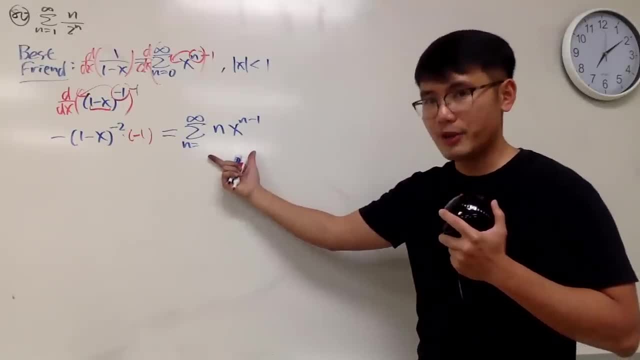 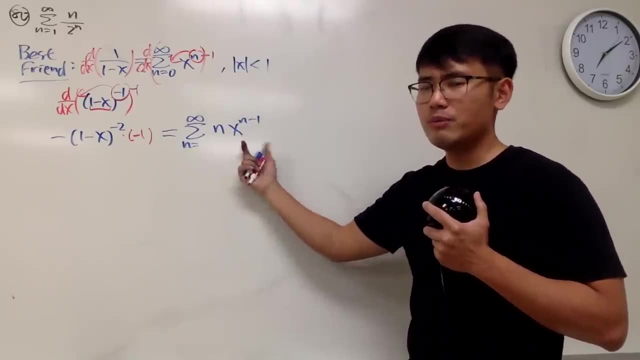 So if you take a look right here, well, if n you just keep it as 0, the first term will be 0. It's okay to have that, but usually when you differentiate, if you lose a term. 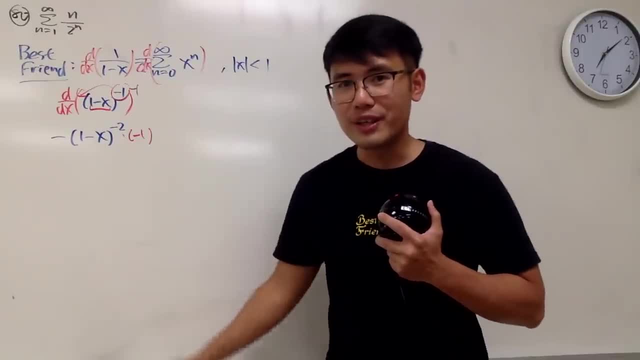 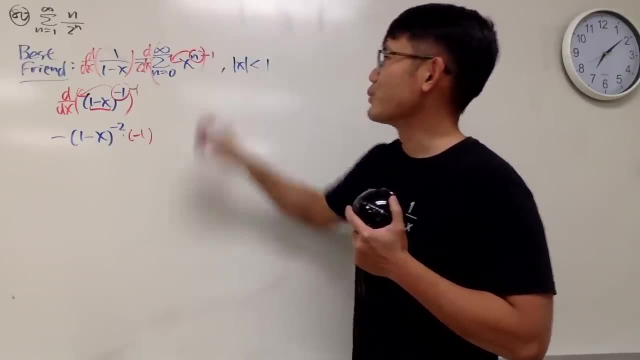 the derivative inside, which is multiplied by negative 1. like this we differentiate this right here. on the left hand side, you just differentiate x to the nth power. bring this to the front minus 1. so let me write this down right here for you guys. this is actually the same as a, the 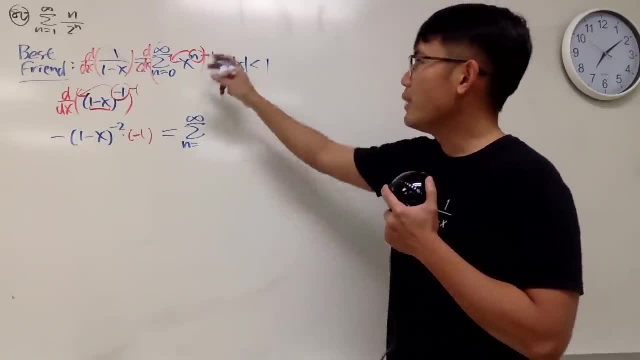 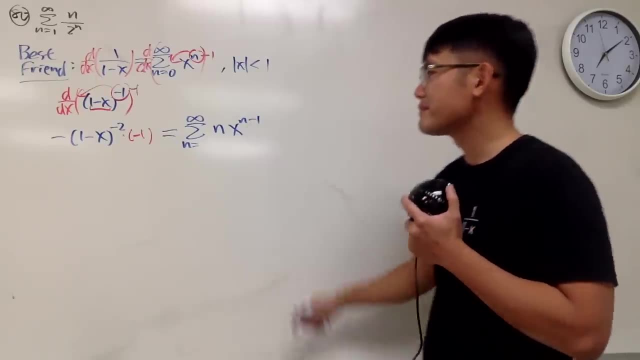 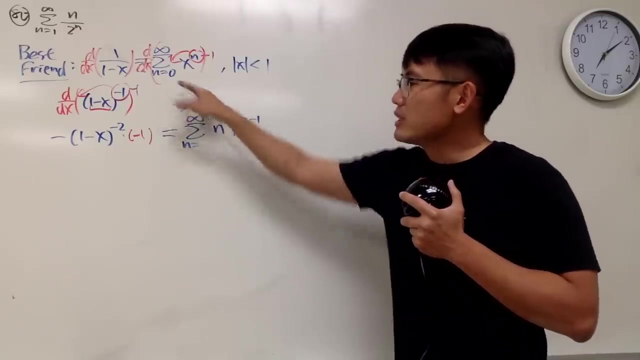 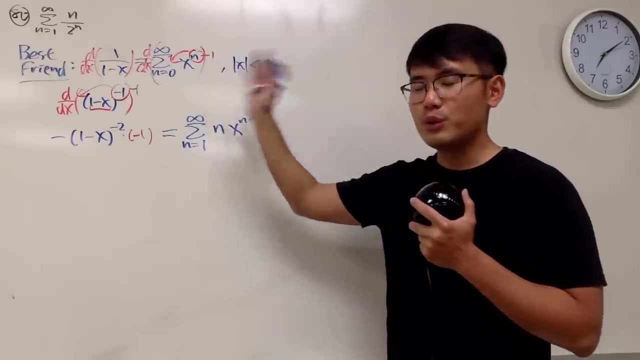 sum as n goes from something to infinity and you have n x to the n minus 1, like this. and now here is the deal, if you take a look right here. well, if n you just keep it as 0, the first time will be 0. it's okay to have that, but usually when you differentiate, if you lose the term. 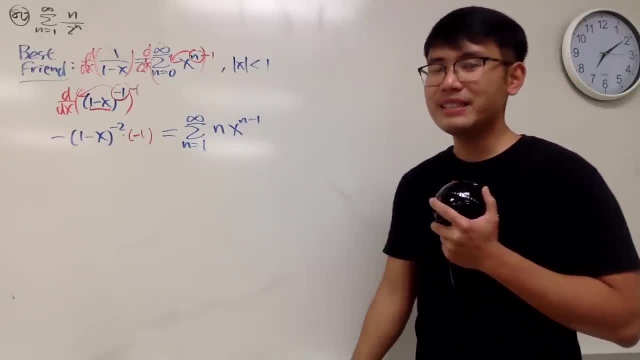 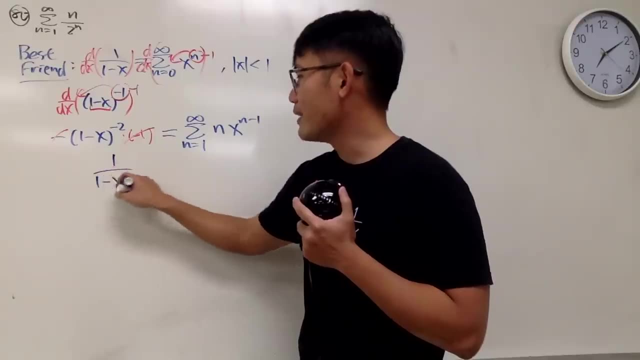 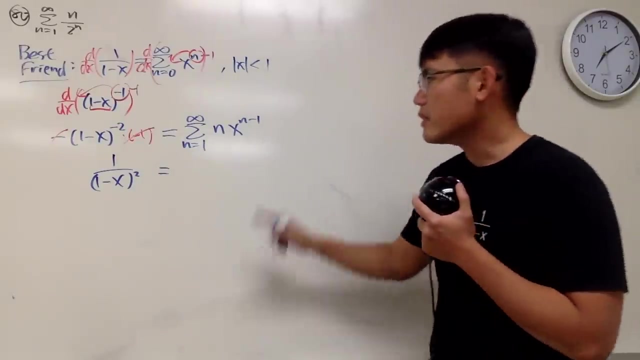 people will just start with: n equals 1, right here. all right now, let's bring up this. and now, of course, they're just positive. and then this right here is just 1 over 1 minus x, and we square that- and- yes, it's on my shirt, by the way- all right now. 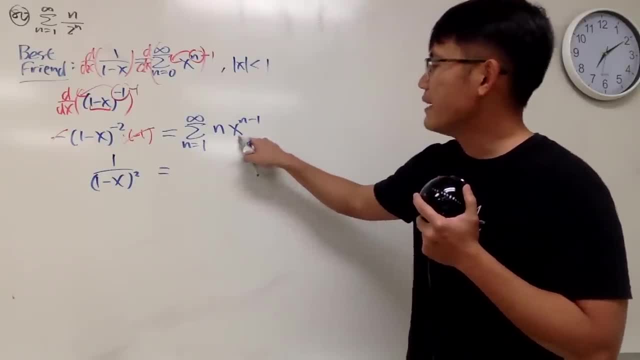 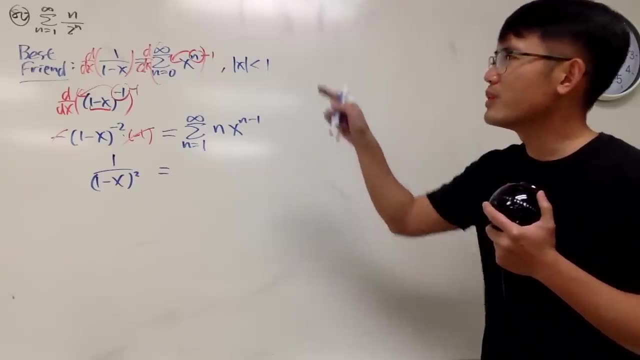 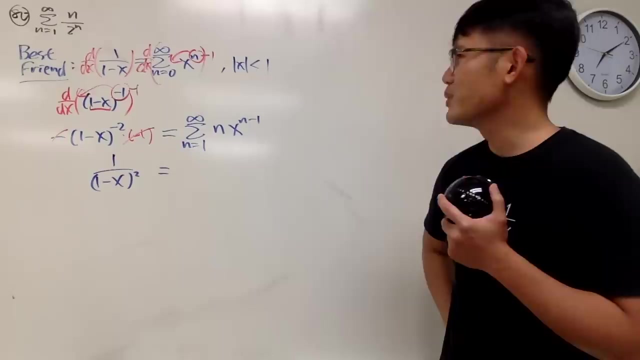 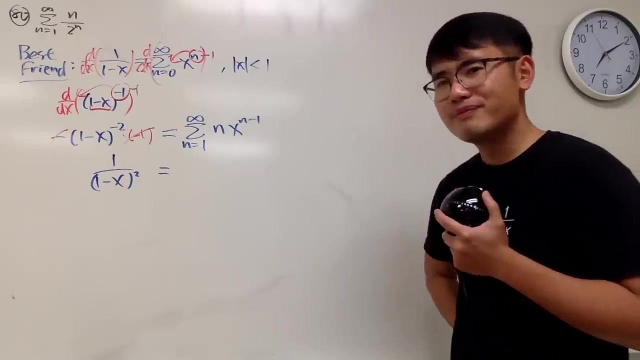 this is another fix. here we have x to the n minus 1. hmm, i kind of want to get to the. i kind of want to get to there. you see, this is 2 to the n. this is x to the n minus 1. let's go ahead and fix. 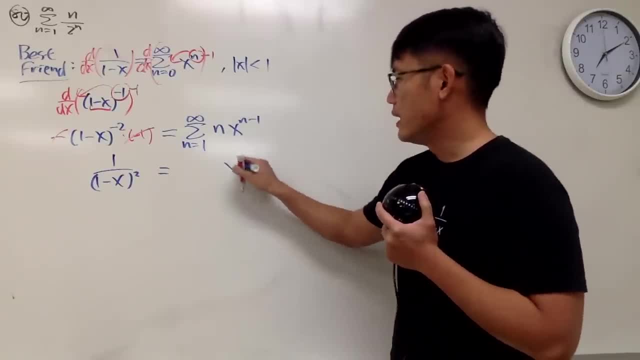 the index a little bit to do. so we do this. x. you're going to add 1, add 1 to the n, so you get n plus 1 minus 1, which is just n, and then you add 1 here, which is n plus 1. so that should be okay and you're. 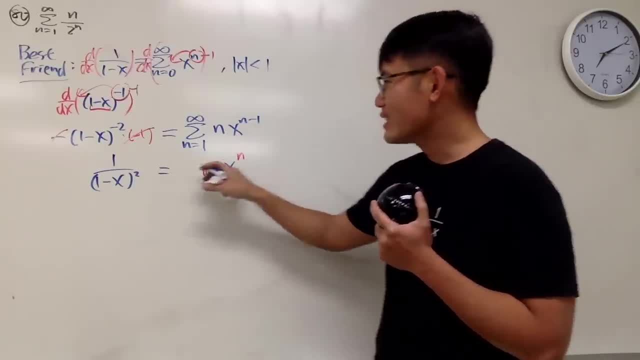 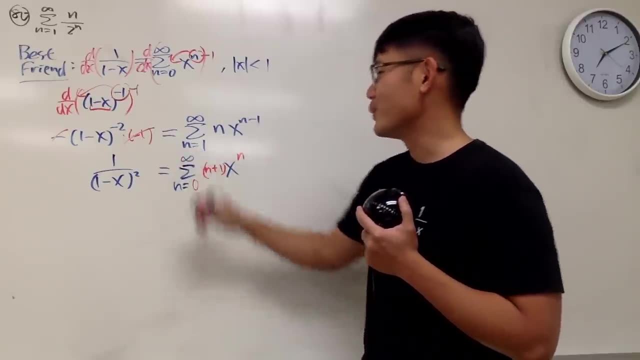 going to subtract 1. subtract 1 right, to just keep things balanced. so you're going to get the sum as n going from 0 again. Yes, I know. And then infinity minus 1 is still infinity, so we're still good. So this is right and this is still true if the absolute value of x is less. 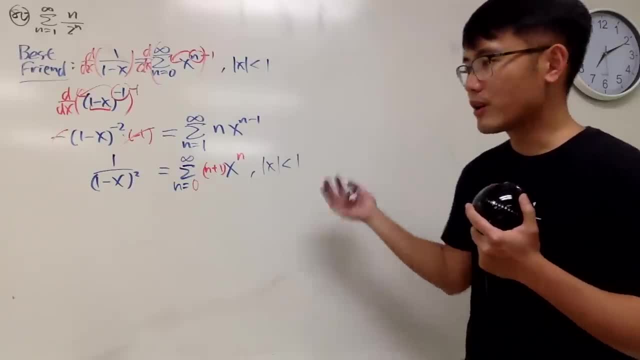 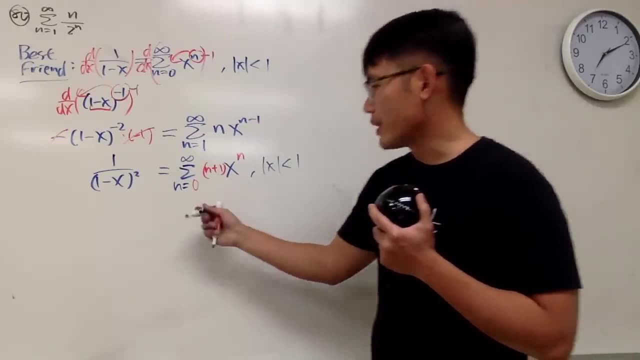 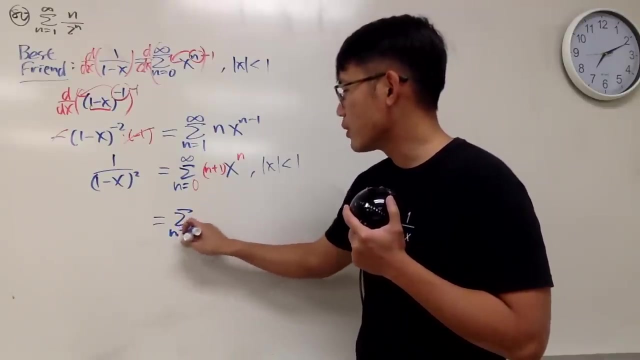 than 1.. It gets trickier if you want to talk about the interval convergence, but maybe that's later on. Anyway, we can do a little bit right here. So if you look at this, we can separate this. This is saying the sum as n going from 0 to infinity, just multiply. 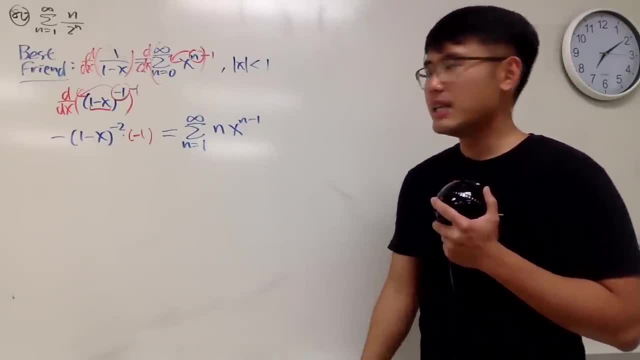 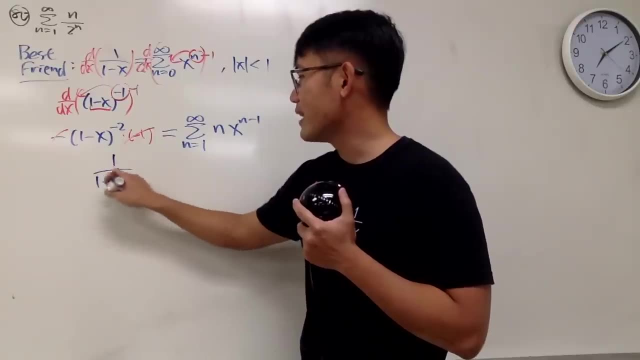 people will just start with n equals 1, right here. alright, Now let's clean up This and that. of course they're just positive. and then this right here is just 1 over 1 minus x, and we square that. and yes, it's on my shirt, by the way- 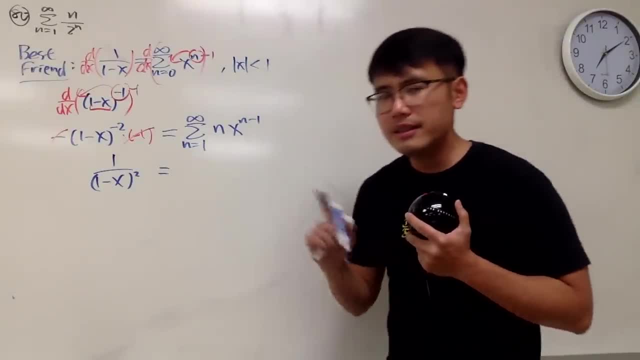 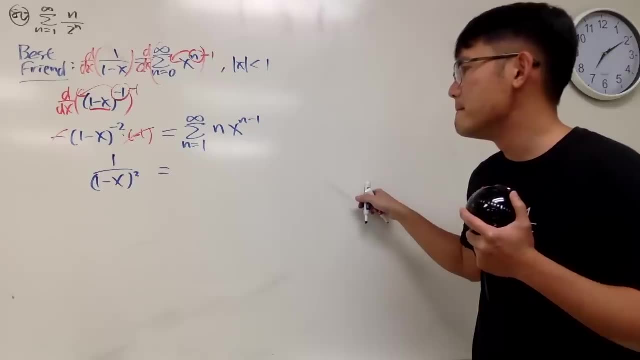 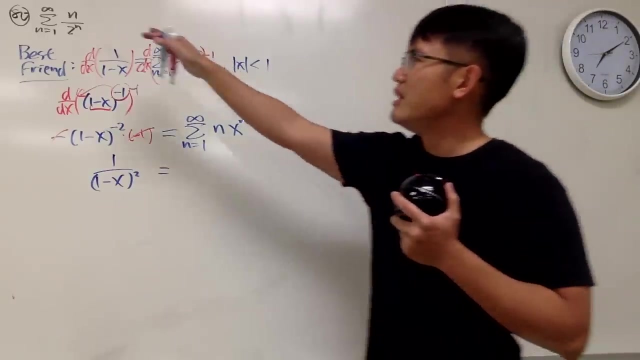 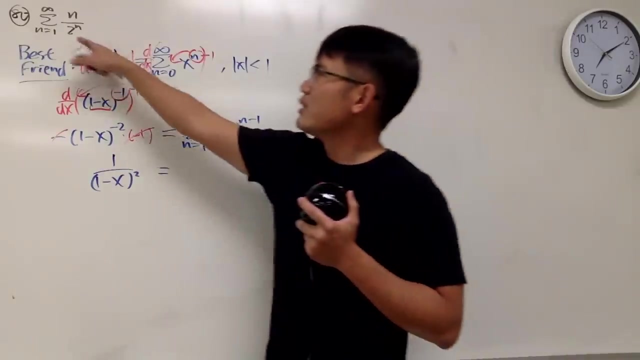 Alright, now this is another fix. Here we have x to the n minus 1.. Hmm, I kind of want to get to the. I kind of want to get to there. You see, this is 2 to the n. this is x to the n minus 1.. 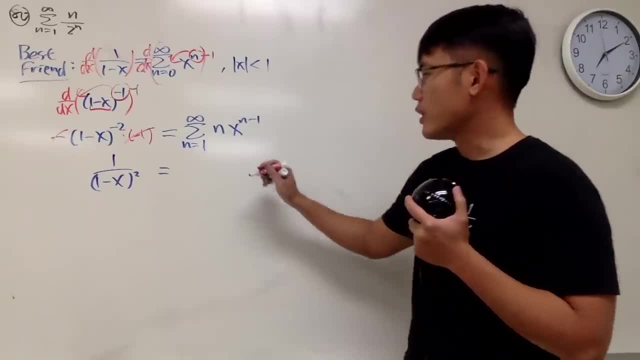 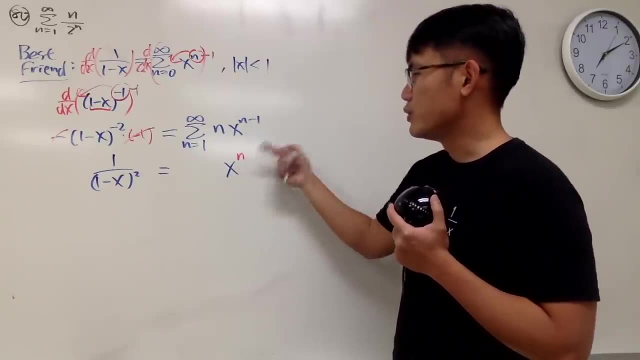 Let's go ahead and fix the index A little bit To do. so we do this: x, You're going to add 1, add 1 to the n so you get n plus 1 minus 1, which is just n. 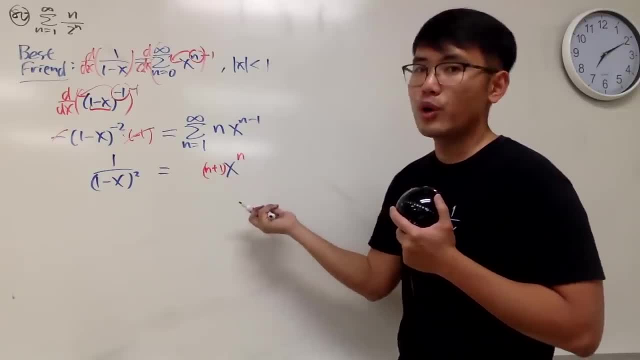 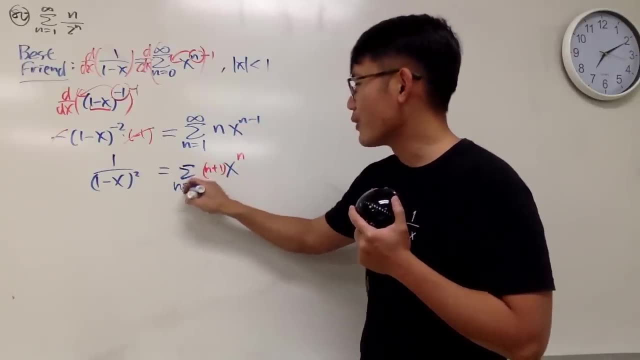 and then you add 1 here, which is n plus 1, so that should be okay. And you're going to subtract 1, subtract 1, right, To just keep things balanced. So you're going to get the sum as n, going from 0 again. 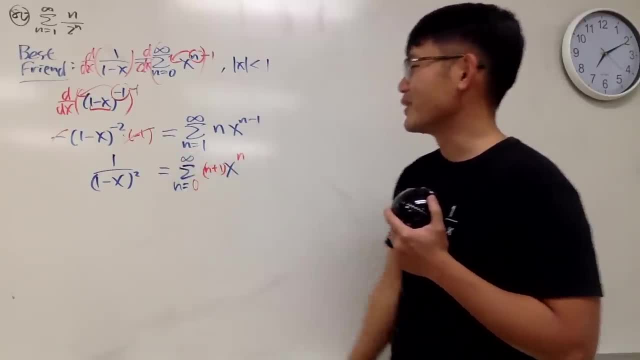 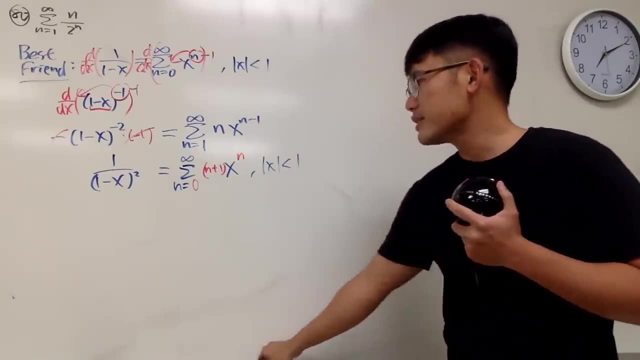 Yes, I know. And then infinity minus 1 is still infinity, so we're still good. So this is right and this is still true if the absolute value of x is less than 1.. It gets trickier if you want to talk about the interval convergence. 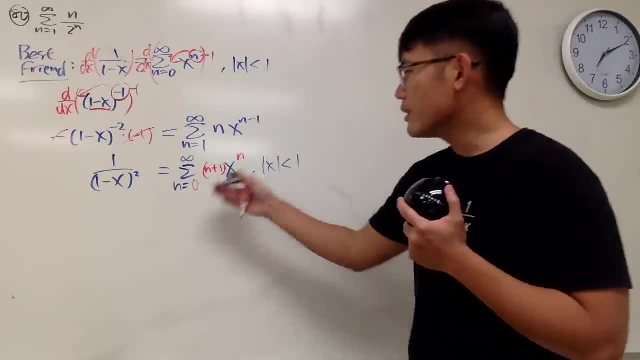 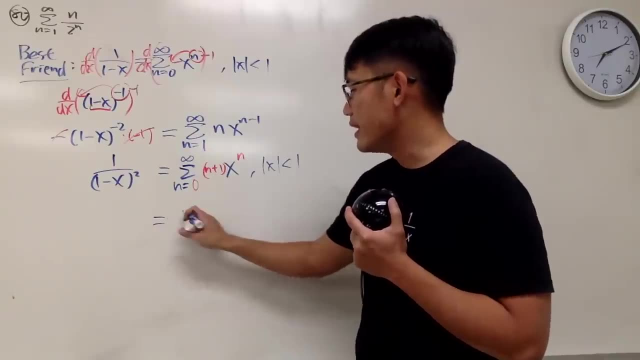 but maybe that's later on. Anyway, we can do a little bit right here, right here, right. So, if you look at this, we can separate this. This is, as I'm saying, the sum as n going from 0 to infinity. 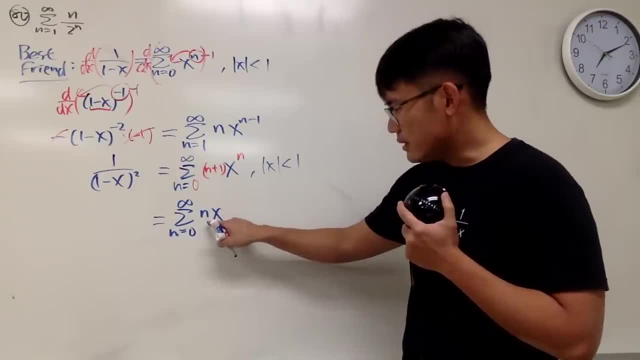 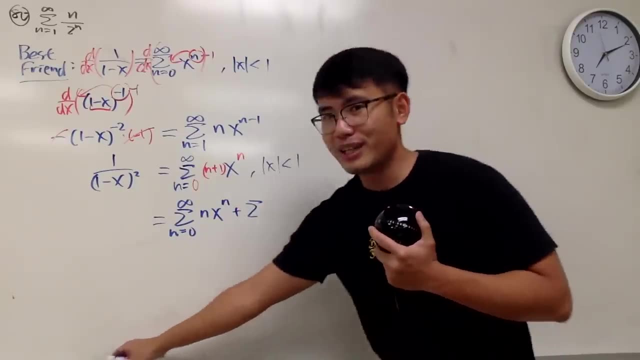 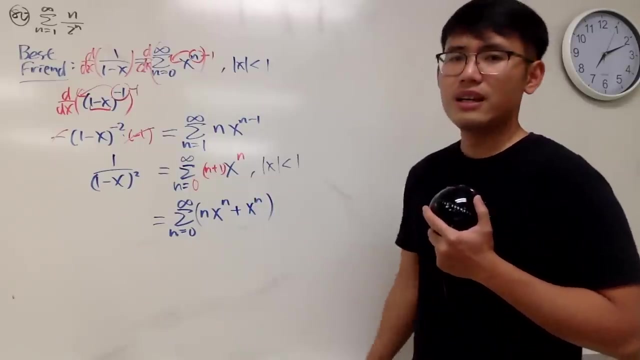 Just multiply it. So the first thing is x to the It's nx to the nth power, and you just add the sum. Well, actually that's true, We can't do that yet. And then you just do this times that which is plus x to the n, like this right. 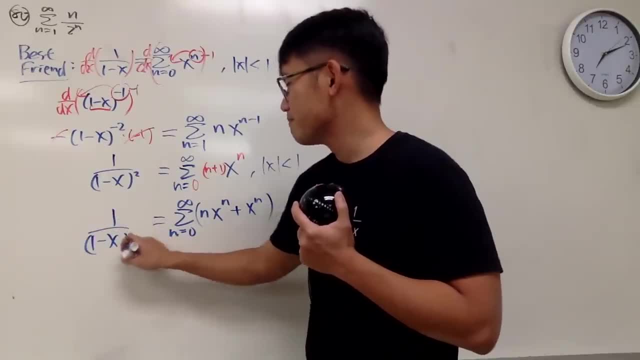 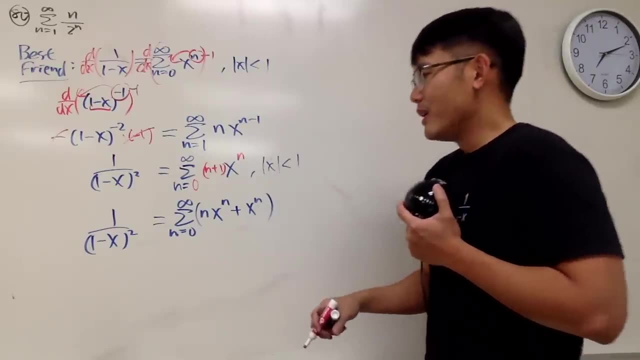 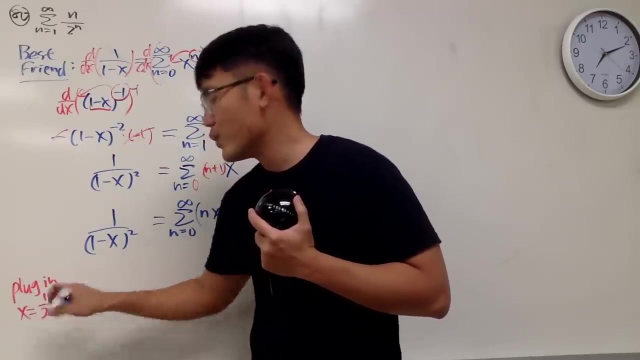 So you have actually a very nice equation like this, And because this is true for n is For, x is less than For, absolute value of x is less than 1, so I'm just going to be plugging: x equals 1 half. 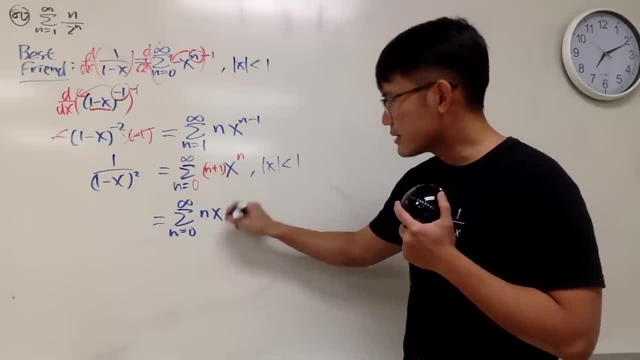 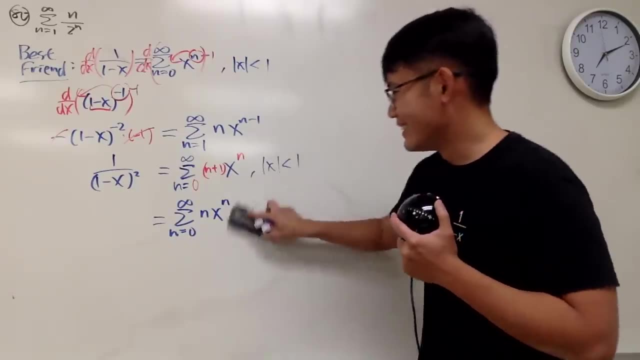 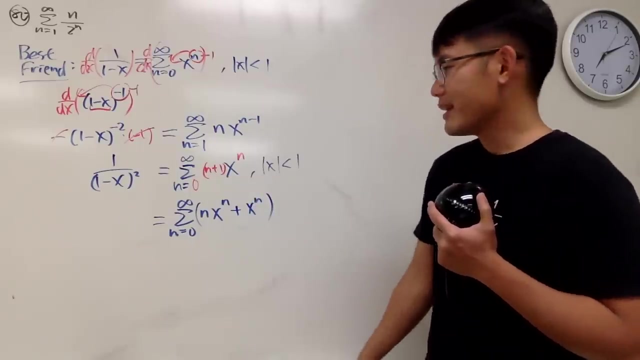 it. So the first thing is nx to the nth power and you just add the sum- Well, actually I shouldn't do that yet- And then you just do this times that which is plus x to the n, like this right. So you have actually a very nice equation like this: 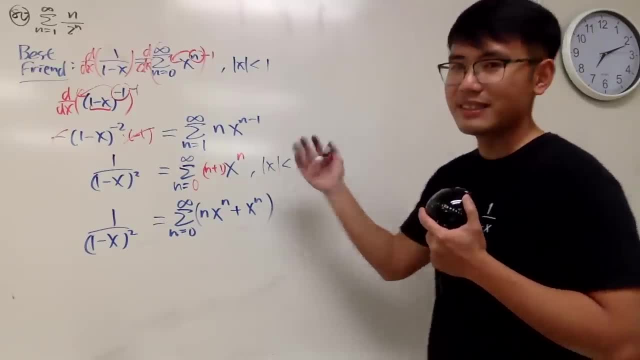 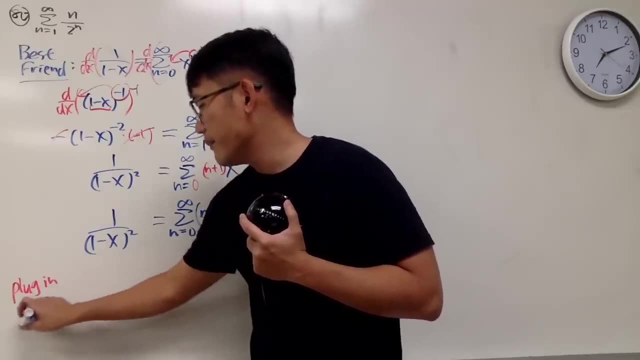 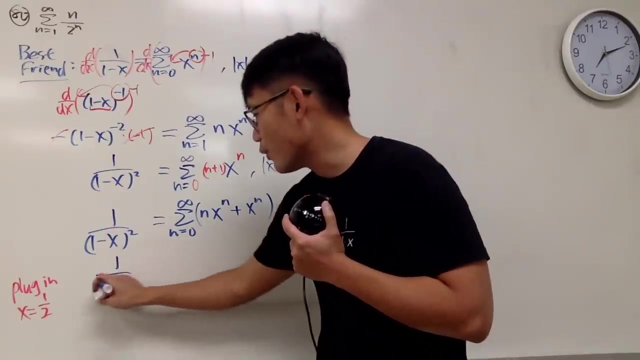 And because this is true for n is for, x is less than for, absolute value of x is less than 1, so I'm just going to be plugging: x equals 1 half. Why? Because I have the 1 half over there And you guys will see that on the left-hand side we have 1 over 1 minus. 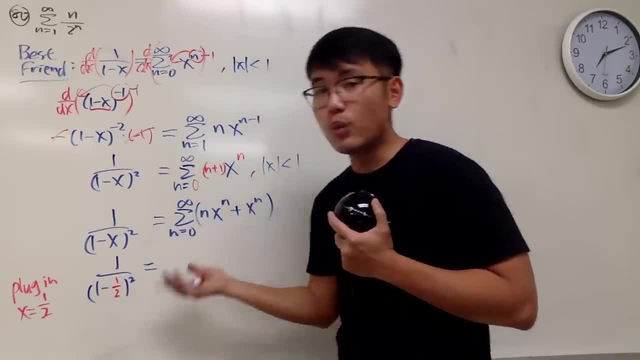 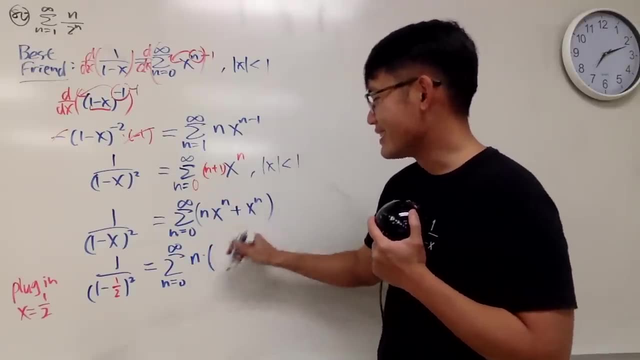 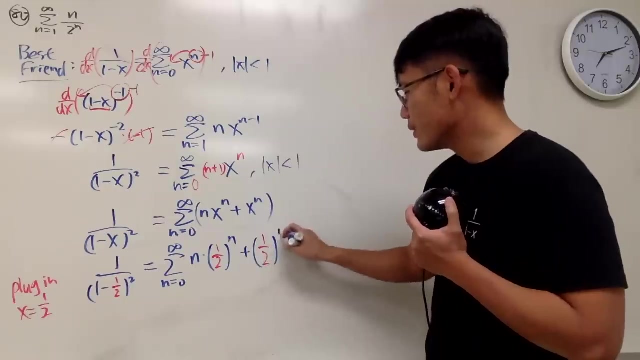 1 half, and we square that This right here will be equal to the sum, as n goes from 0 to infinity. This is n times. yes, we get the 1 half, 1 half to the nth power. And then here we have plus 1 half to the nth power, like this: 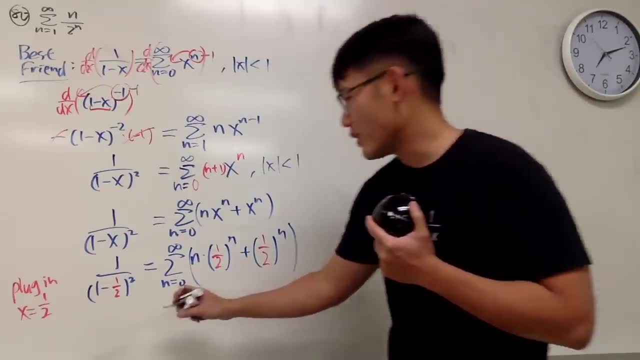 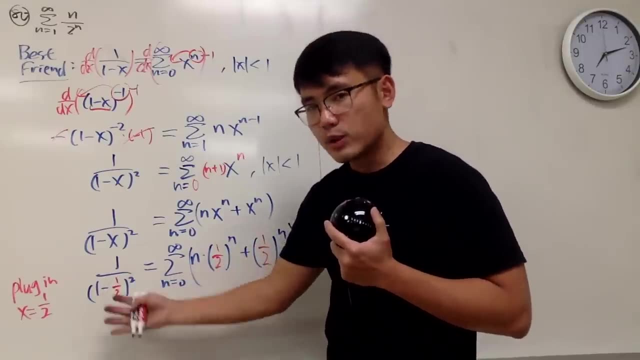 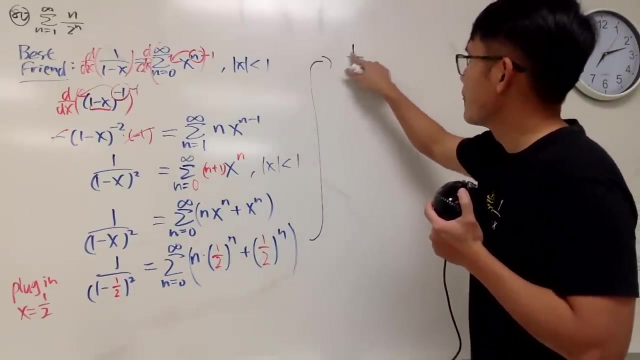 Okay, this is exactly what we're trying to get, So I will just write this down right here for you guys. The left-hand side. let's do this in your head: This is 1 half square, which is 1 over 4 in the denominator. so we get 1 over, we get positive 4 on the left-hand. 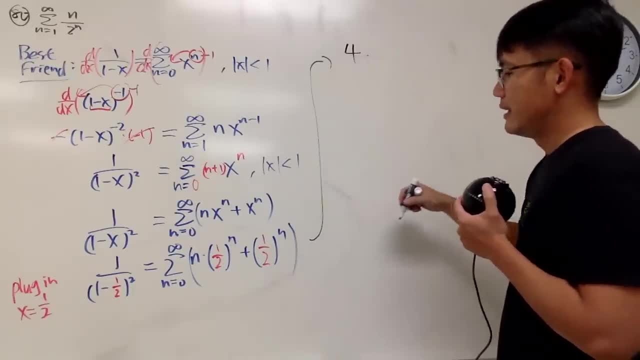 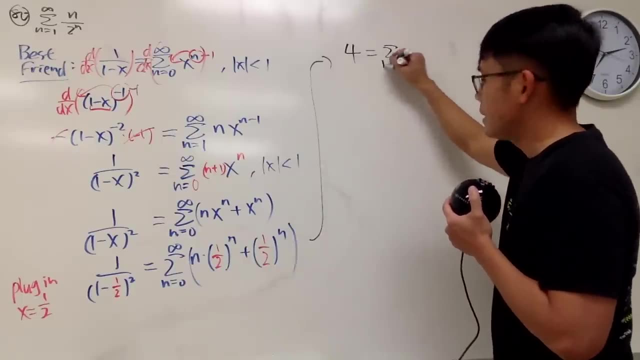 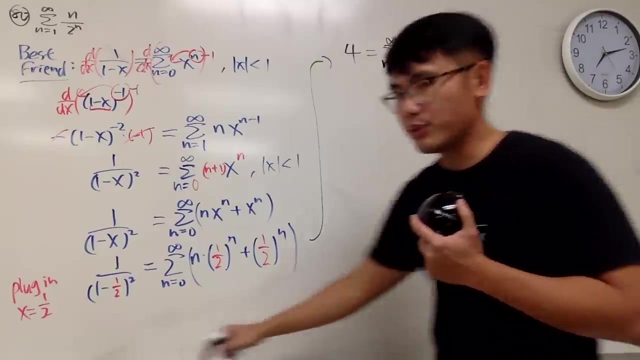 side. We just square that and all that. Okay, Here is equal to. let me just kind of look at this sum and that sum individually. we know this is the sum, as n goes from 0 to infinity, and I will just put it down right here, to save some space. You can look at the sum of: 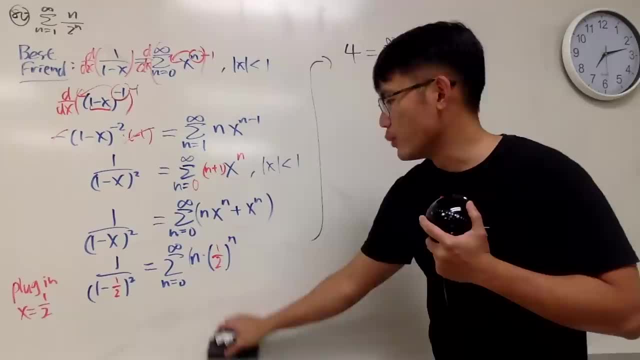 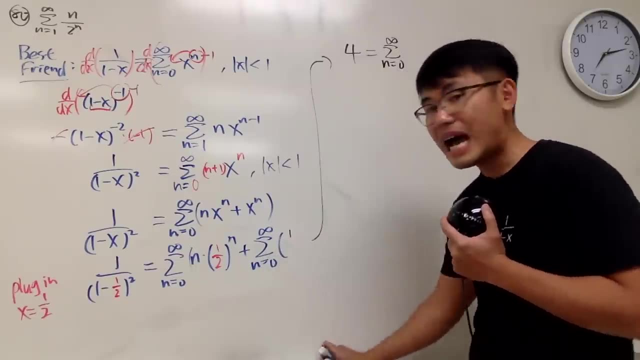 this and also the sum of that. So I will just tell you it works like integral. You can look at plus the sum, as n goes from 0 to infinity. parentheses: 1 half- Right, Because x is 1 half, Okay. 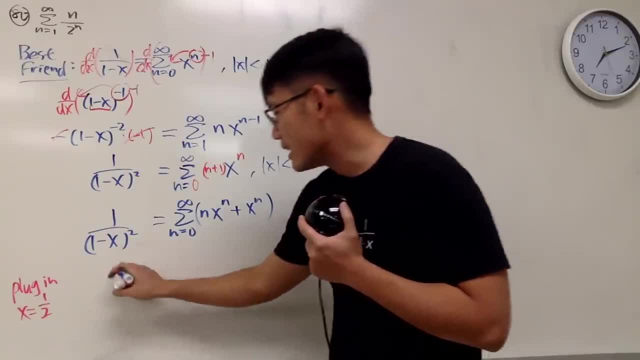 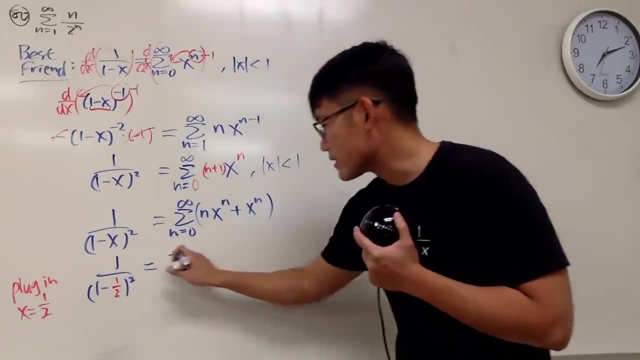 Why? Because I have the 1 half over there And you guys will see that On the left-hand side we have 1 over 1 minus 1 half And we square that This right here will be equal to the sum, as n goes from 0 to infinity. 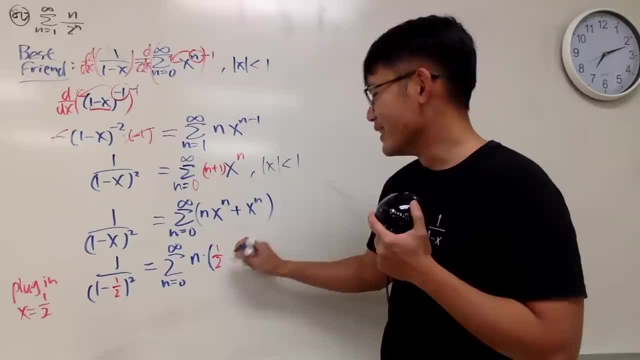 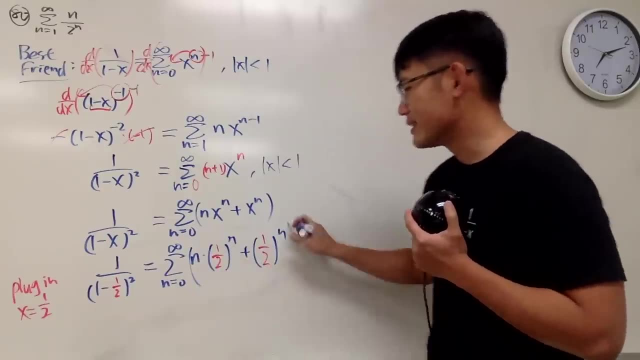 This is n times. Yes, we get the 1 half to the nth power, And then here we have plus 1 half to the nth power, like this: Okay, This is exactly what we're trying to get, So I will just write this down right here for you guys. 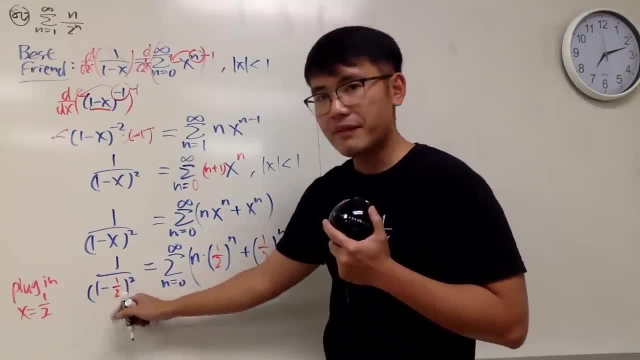 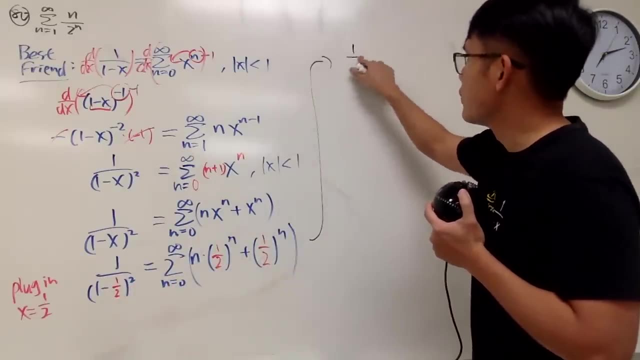 The left-hand side. Let's do this in your head: This is 1 half squared, which is 1 over 4 in the denominator. So we get 1 over, We get positive 4 on the left-hand side. We just square that and all that. 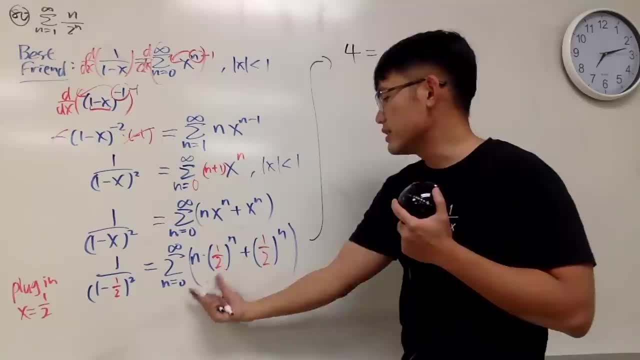 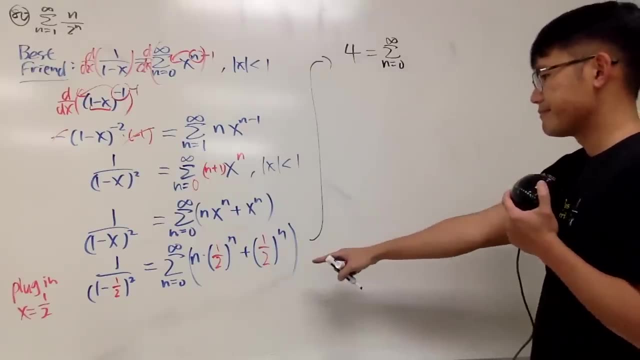 Here is equal to. Let me just kind of look at this sum and that sum individually. We know this is the sum, as n goes from 0 to infinity, And I will just put it down right here to save some space. You can look at the sum of this and also the sum of that. 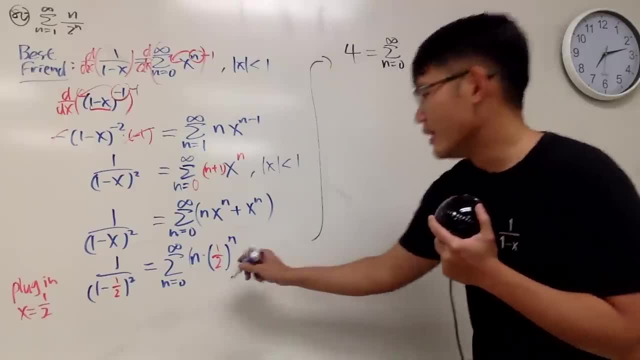 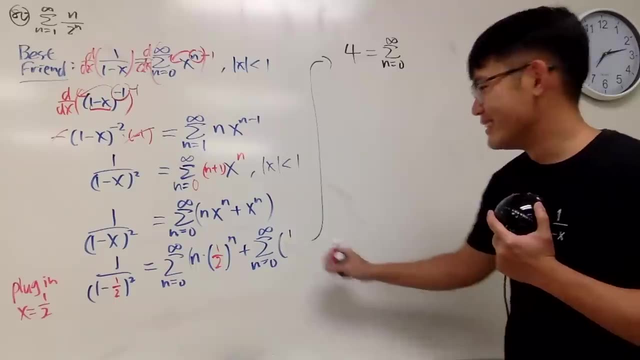 So I will just tell you It works like integral. You can look at plus the sum as n goes from 0 to infinity- parenthesis: 1 half Right, Because x is 1 half Right here- And then raise that to the nth power. 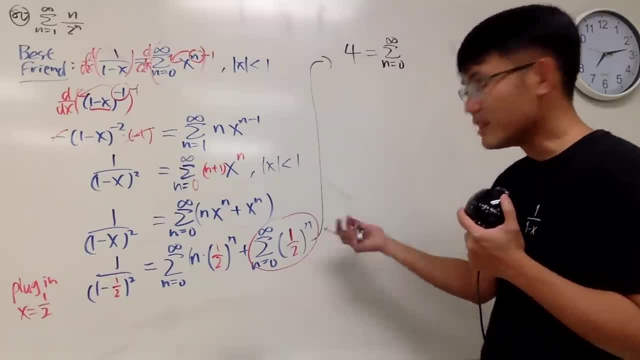 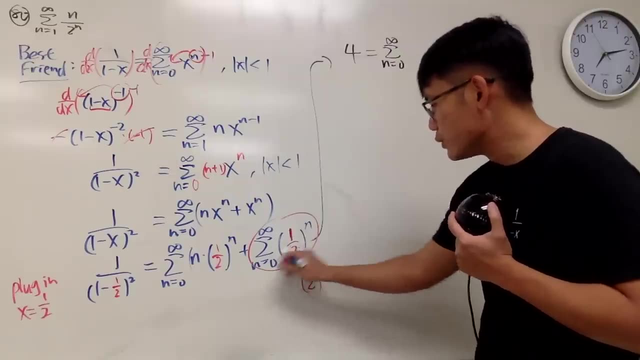 And the beauty of this is that we can use our best friend to help us out. This right here is actually equal to the first term, So it's 1 half raised to the 0th power, Divided by 1 minus the common ratio, which is 1 half. 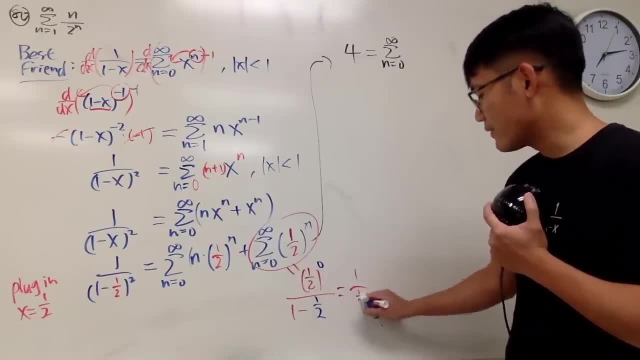 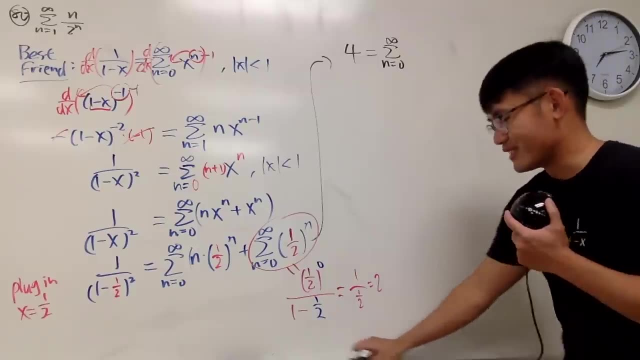 Here we get 1 over 1 half, which is 2.. So in fact, this right here will give us 2.. But I forgot to write that down, so I will write that down first. I will put this down as n. 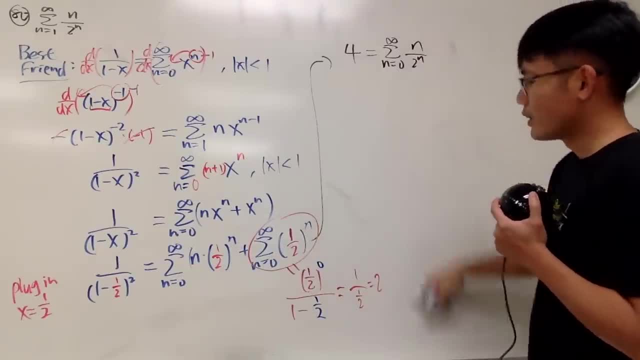 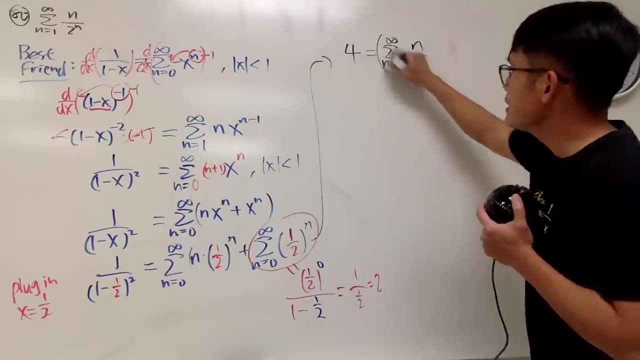 And then 1 to the nth is just 1.. And then we have over 2 to the nth power, And this right here is just 2.. So we have This thing And then in the end we add a 2 to it. 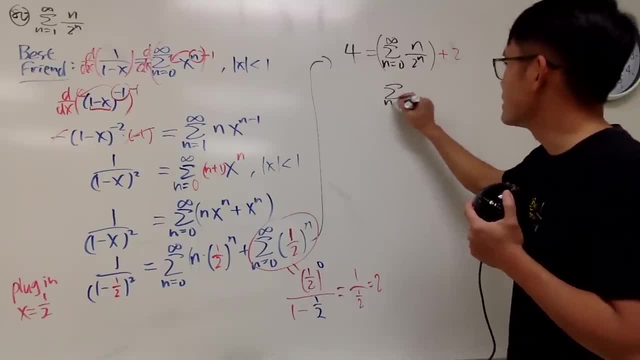 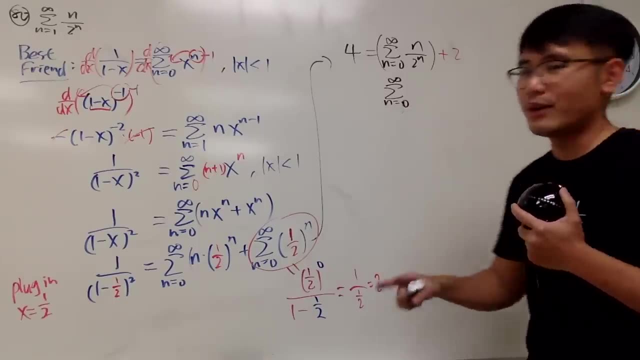 Oh my god, Minus 2 on both sides. Finally, we can say: the sum as n goes from 0 to infinity. Okay, This is going from 0 to infinity. Okay, I know, I know. Hmm, Oh, that was overkill. 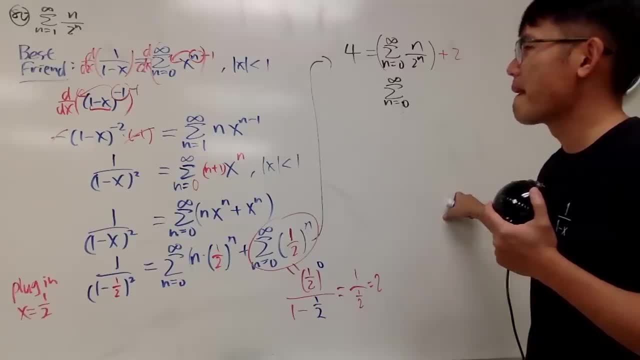 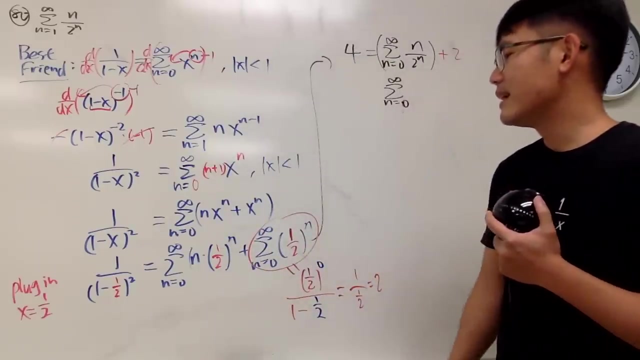 Oh, my god, I didn't pay attention to that thing. Oh, I could have just done the 1 half right here instead of doing all this. Um, yeah, because I was thinking about doing the differential equation. So if you want to continue right here, that's fine. 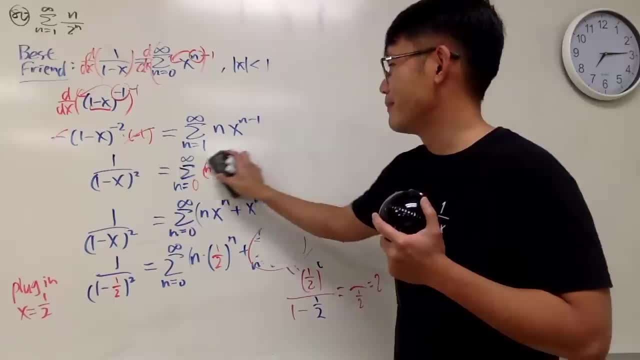 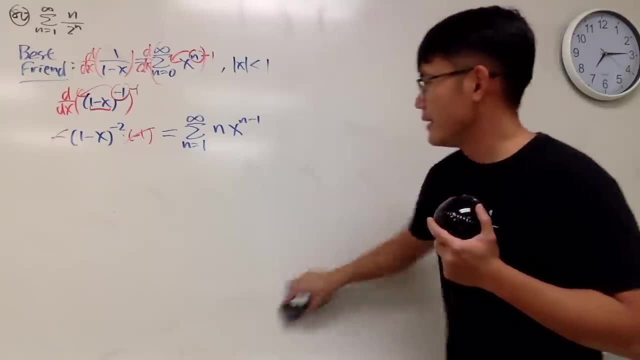 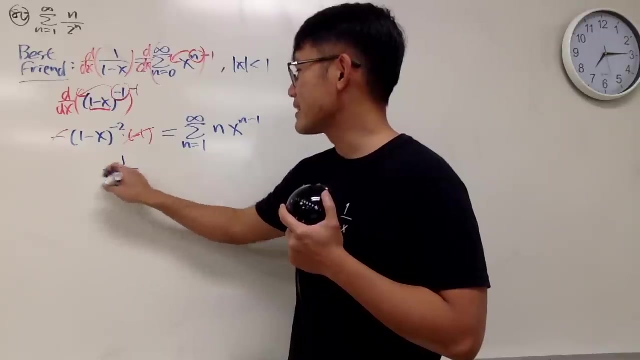 But like this is not necessary, So just skip to here, I would say: Okay, Anyway, right here on the left-hand side, we have this as 1 over 1 minus x squared. Yeah, The right-hand side. 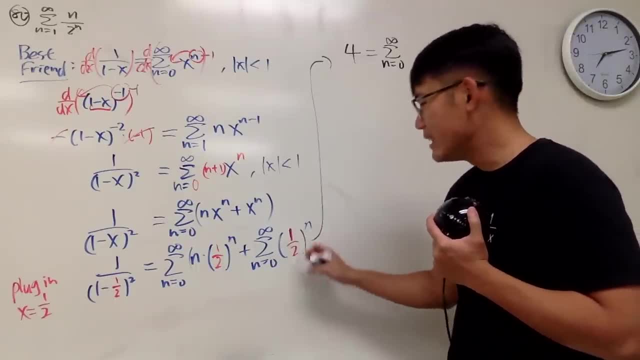 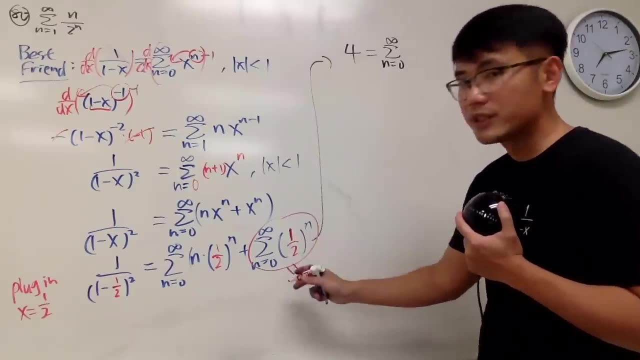 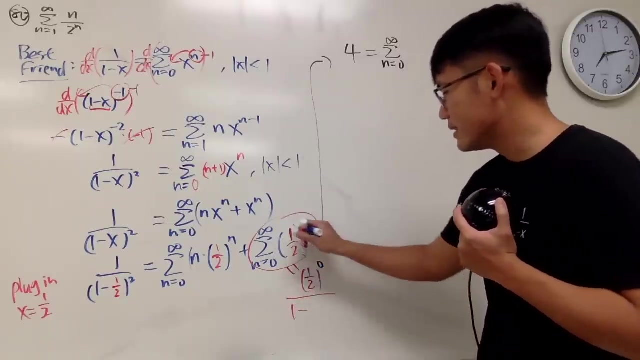 right here and then raise that to the nth power, And the beauty of this is that we can use our best friend to help us out. This right here is actually equal to the first term. is 1 half raised to the 0th power divided by 1 minus the common ratio, which is 1 half. 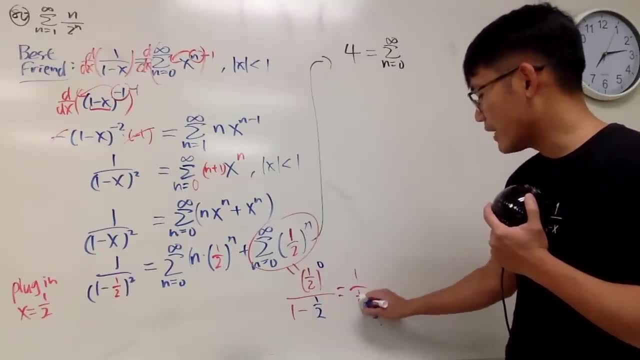 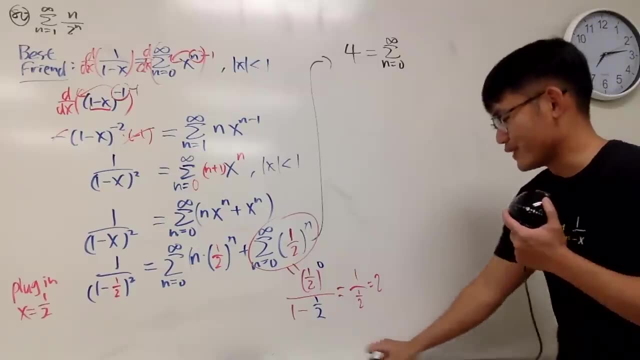 Here we get 1 over 1 half, which is 2.. So in fact this right here will give us 2, but I forgot to write that down, so I will write that down. first I will put this down as n, and then 1 to the nth is just 1,. 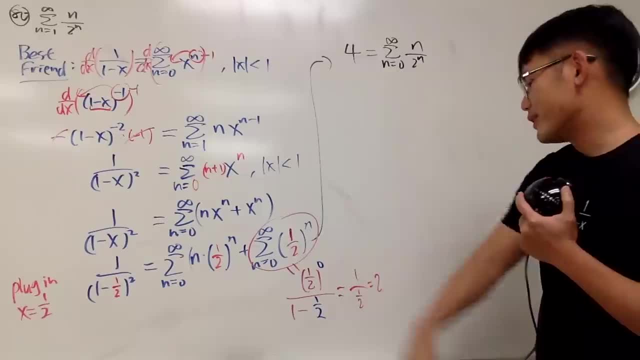 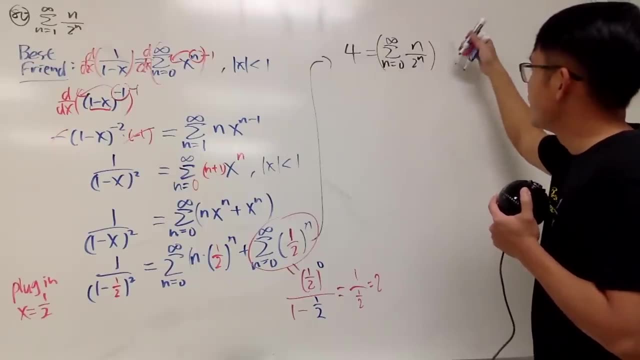 and then we have over 2 to the nth power, and this right here is just 2.. So we have this thing and then in the end we add a 2 to it. Oh my god, minus 2 on both sides. 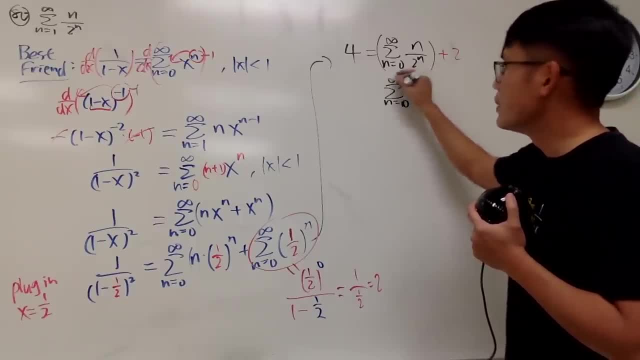 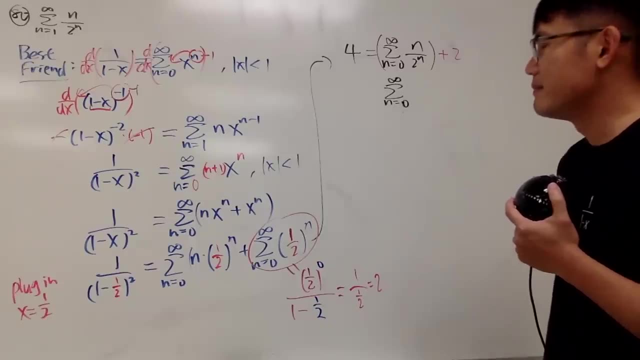 Finally, we can say the sum as n goes from 0 to infinity. Okay, this is going from 0 to infinity. Okay, I know, I know. Hmm, Oh, that was overkill. Oh, my god, I didn't pay attention to that thing. 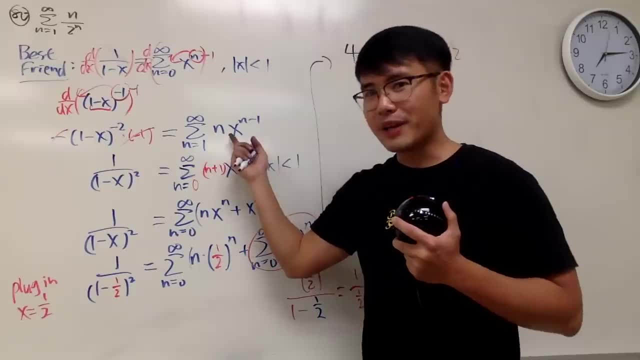 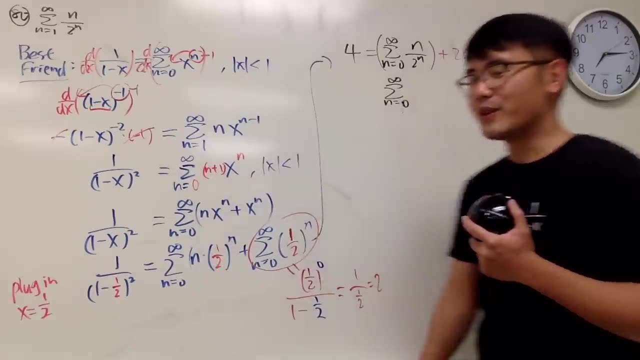 Oh, I could have just done the 1 half right here instead of doing all this. Yeah, because I was thinking about doing the differential equation. so if you want to connect, you can do it right here. that's fine, but like this is not necessary. 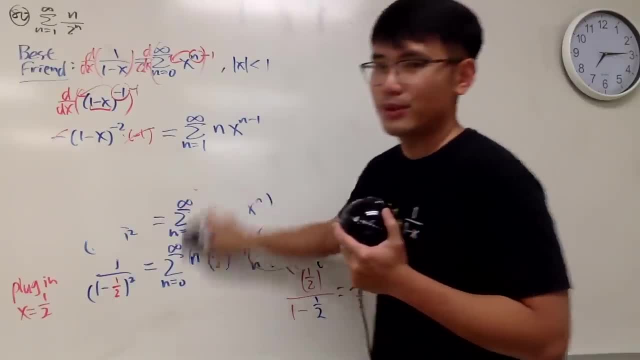 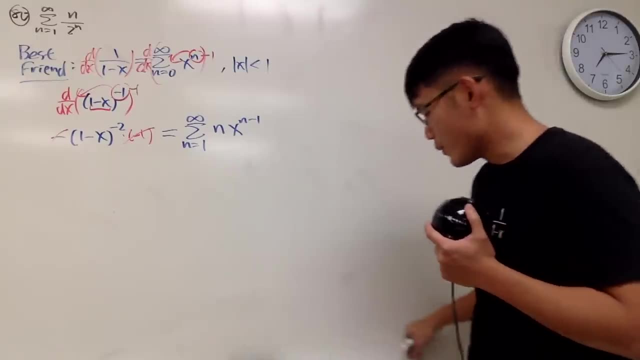 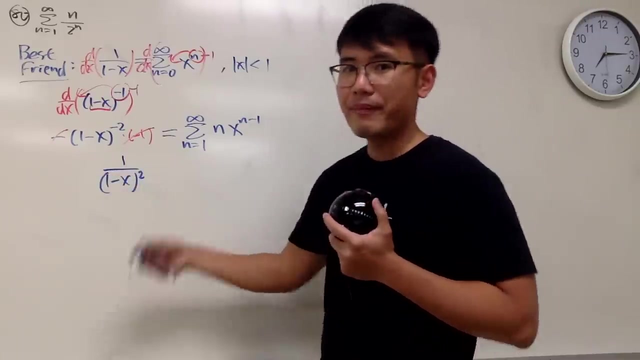 so just skip to here. I would say: Okay anyway, right here on the left-hand side, we have this as 1 over 1 minus x squared. yeah, The right-hand side. check this out, We know this right here. it will actually still be true. 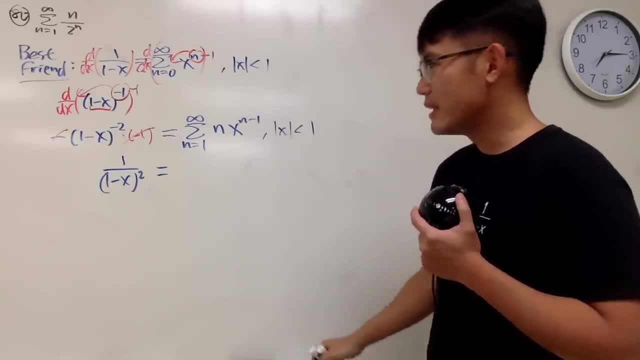 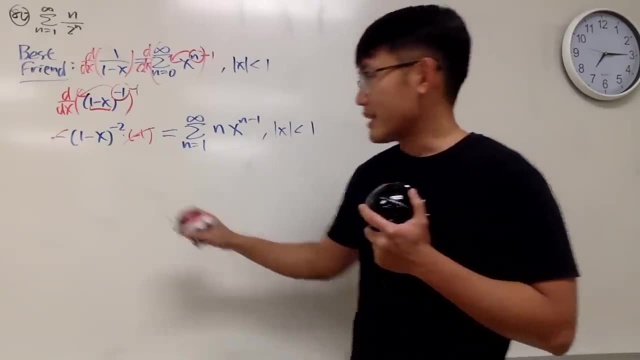 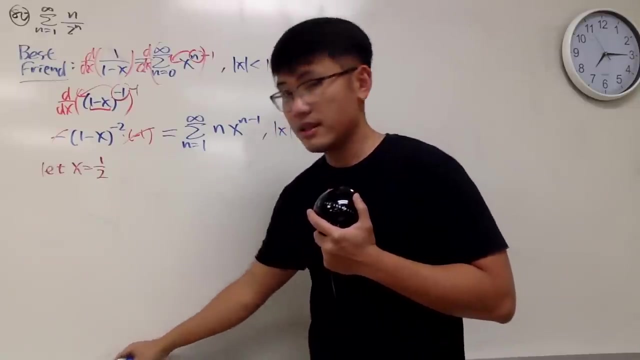 if the absolute value of x is less than 1, right. So the deal is that I will actually write it down right here for you guys. I will plug in that x equal to 1 half, right here. And when we do that on the left-hand side, we get 1 over 1 minus 1 half. 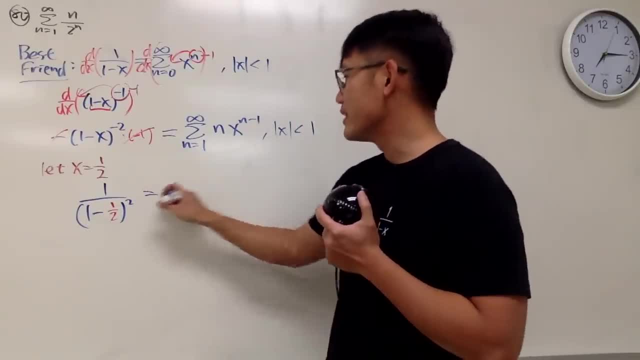 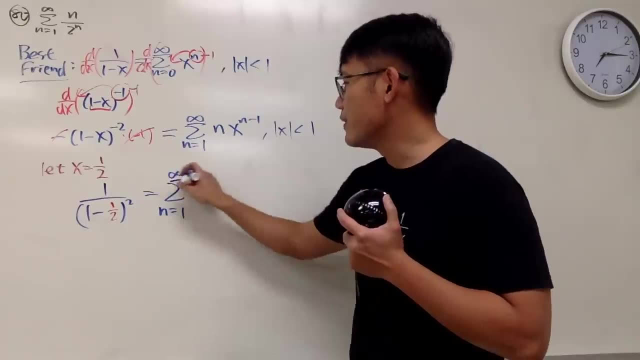 and we square that and then on the right-hand side we actually end up with: n goes from 1 to infinity. So I wasn't paying attention to that, But anyway, n goes from 1.. n goes from 1 to infinity. n is n. 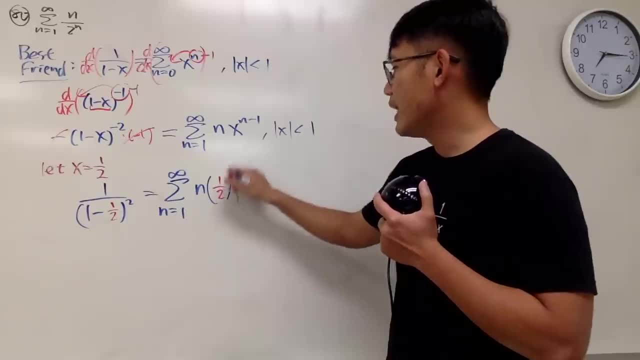 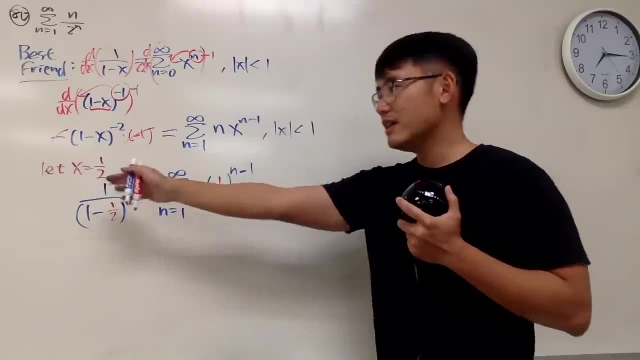 and we're just putting 1 half right here, so which is 1 half, And we have n minus 1, like this, This converges because we have this criteria right And x is just 1 half, which satisfies this. 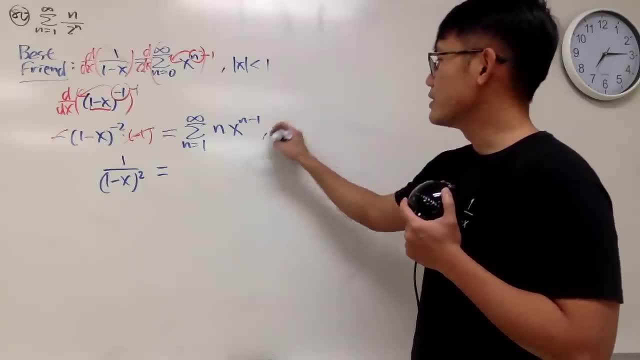 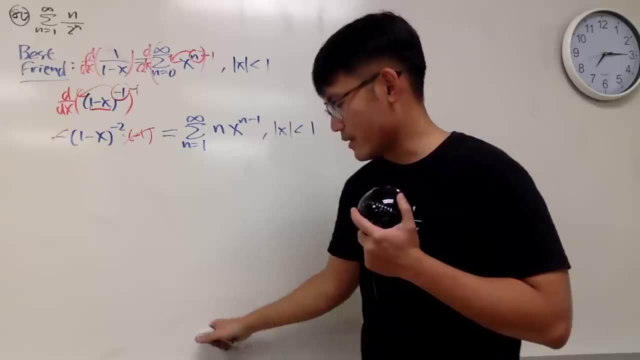 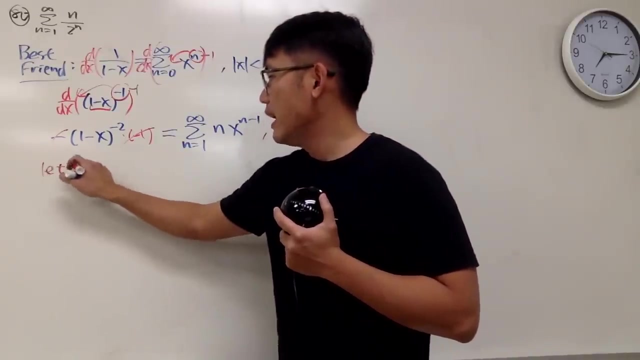 Check this out. We know this right here: it will actually still be true if the value of x is less than 1.. Right, So the deal is that I will actually write it down right here for you guys. I will plug in that x equal to 1 half. 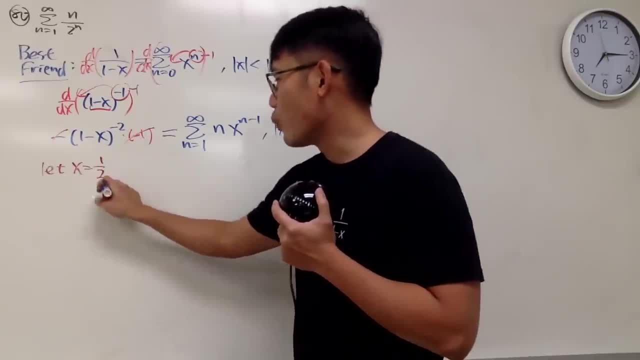 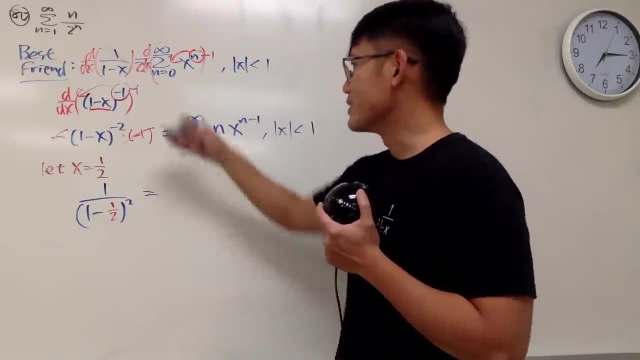 Right here, Right here. So if we do that, on the left-hand side we get 1 over 1 minus 1 half and we square that and then on the right-hand side we actually end up with c. 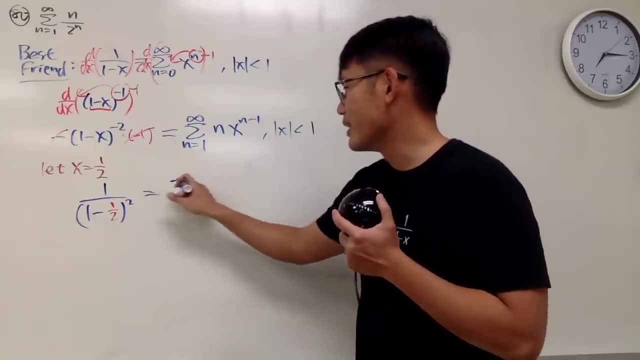 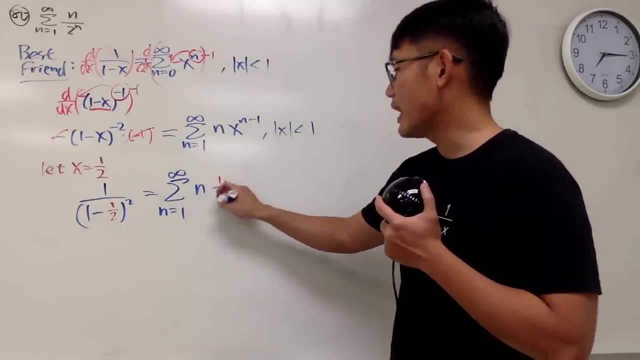 n goes from 1 to infinity, so I wasn't paying attention to it, But anyway, n goes from 1 to infinity. n is n and we're just putting 1 half right here, so which is 1 half, and we have n minus 1, like this: 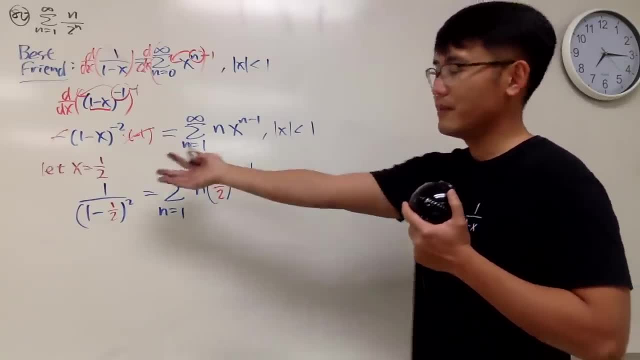 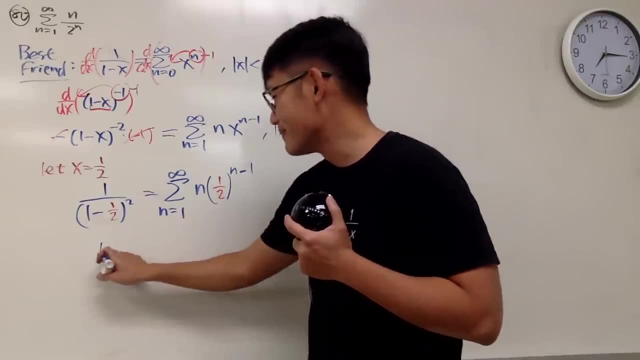 This converges because we have this criteria right And x is just 1 half, which is it's just a regular 2. Now, of course, this right here gives you 4. This right here. Hmm, Let's see. 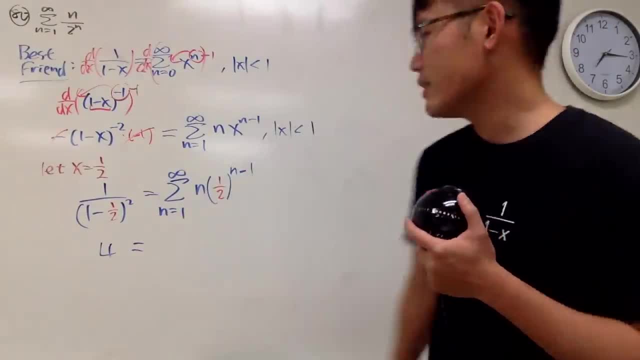 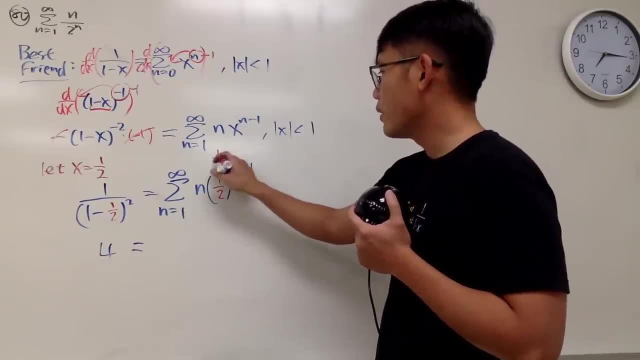 I think earlier did I do the 1 or did I do the? Oh, I did the 1 as well, so that's nice, Okay. So this right here, it's the same as saying 1 over 2 to the n times 1 over 2 to the negative 1.. 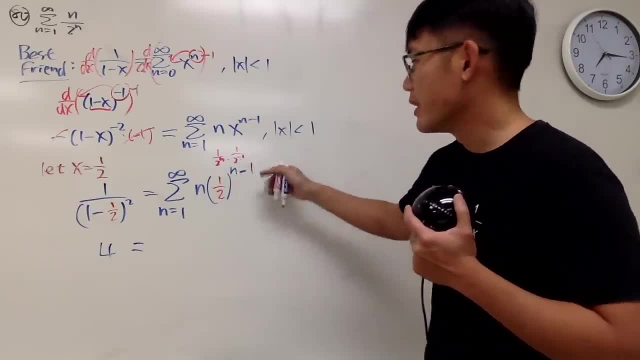 Right If you play along with the power. So this right here is just a regular 2.. So this right here is just a regular 2.. So this right here is just a regular 2.. regular 2, I'll put it down like this and then multiply by the sum as n goes from 1. 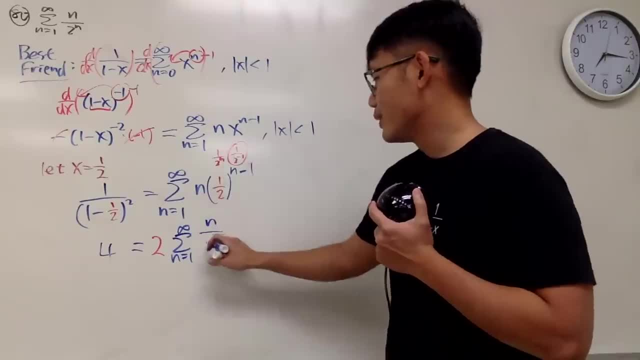 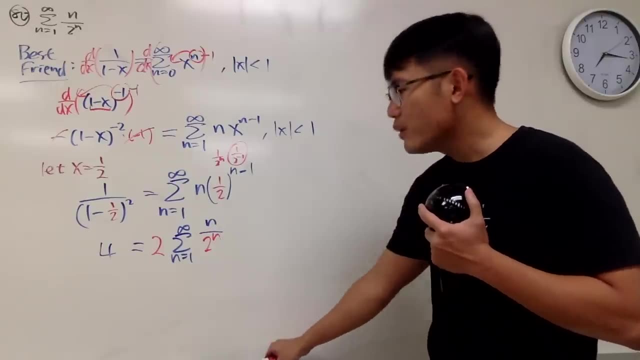 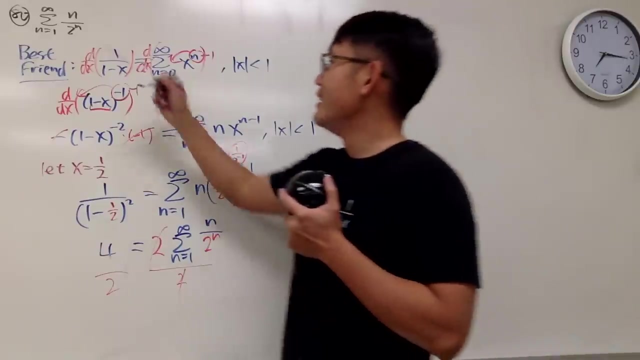 to infinity and we have n over 2 to the n right here. I'll just play along with this and, depending on how much algebra you want to show, finally divide both sides by 2.. Of course, divide both sides by 2, let me just show you guys that Done, So this right. 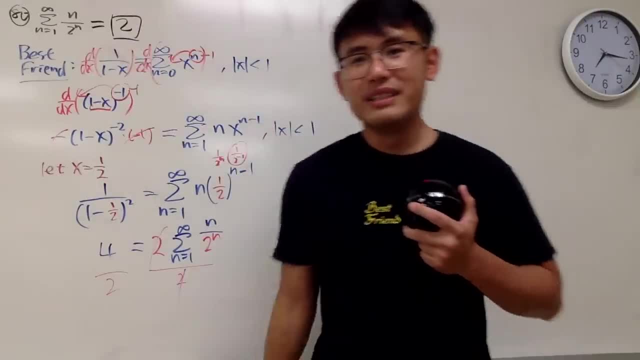 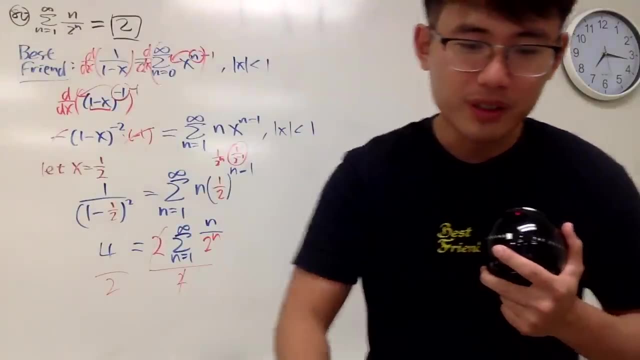 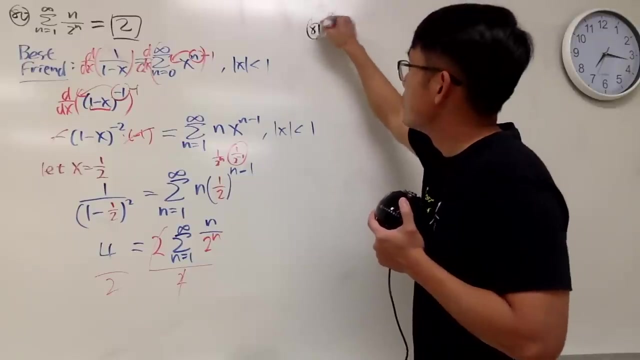 here converges to 2,, thanks to our best friend, actually the derivative version of that. Now here are some of the weirder questions. We'll see number, which is number 90, but we are not there yet. Okay, So we will be asking for what value so that the series will. 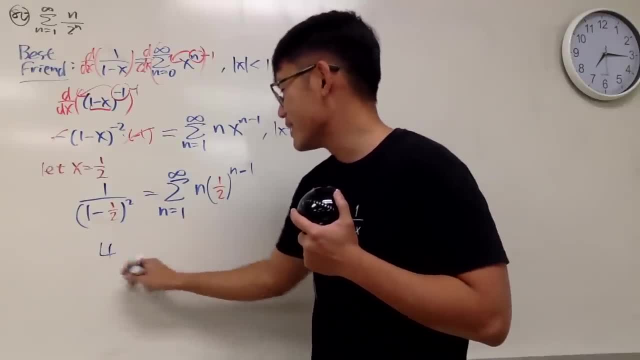 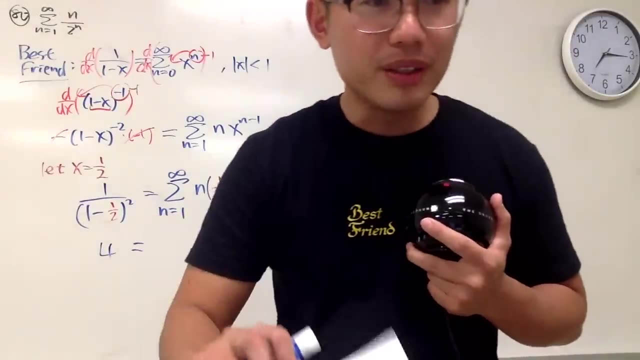 Now, of course, this right here gives you 4.. This right here, hmm, let's see, I think earlier did I do the 1? What did I do? Oh, I did the 1 as well, so that was nice. 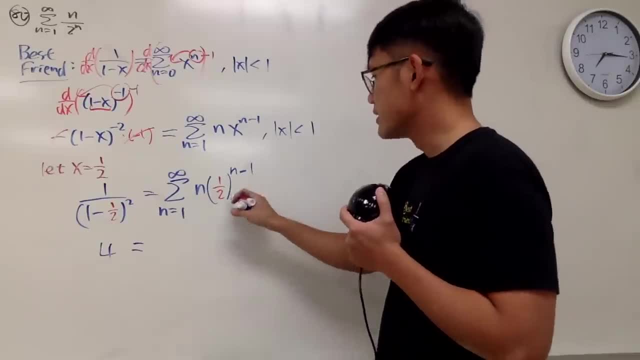 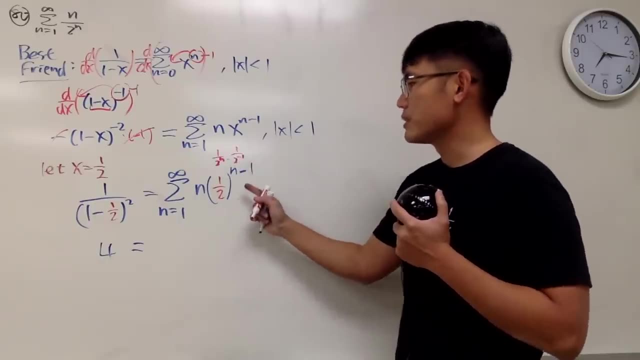 Okay. so this right here it's the same as saying 1 over 2 to the n times, 1 over 2 to the negative, 1, right If you play along with the power. So this right here is just a regular 2.. 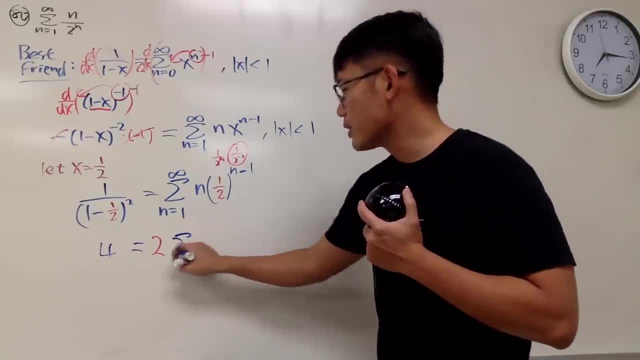 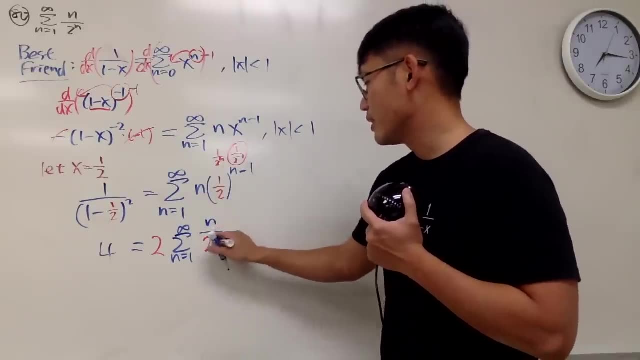 So this right here is just a regular 2.. I'll put it down like this and then multiply by the sum, as n goes from 1 to infinity and we have n over 2 to the n right here. I'll just play along with this and depending on how much algebra you want to show, 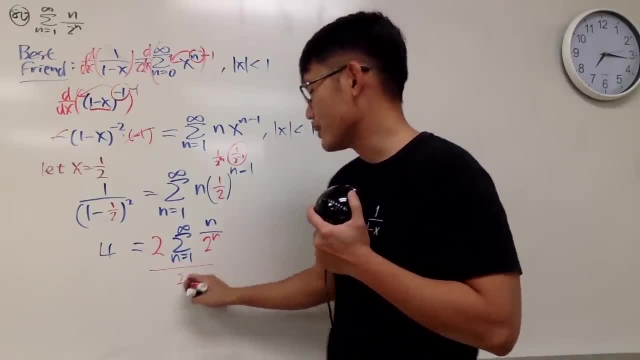 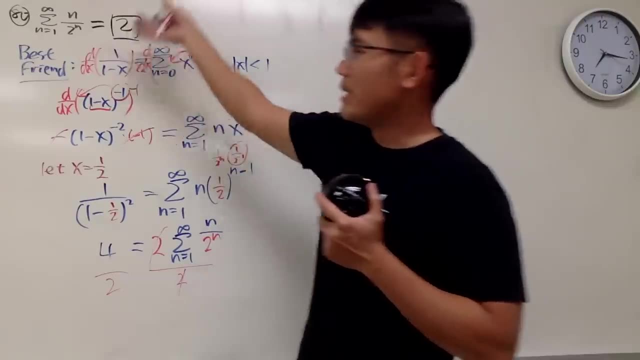 Finally divide both sides by 2,, of course, divide both sides by 2.. Let me just show you guys that Done. So this right here converges to 2, thanks to our best friend, Actually, the derivative version of that. 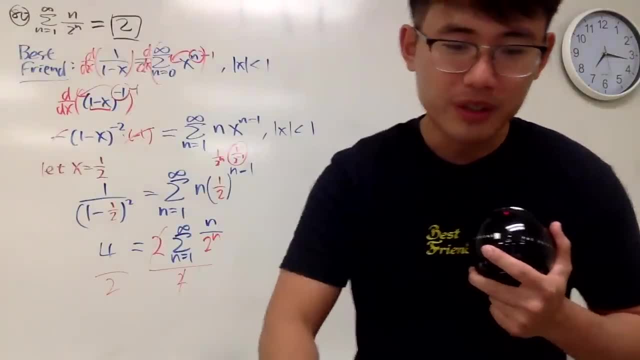 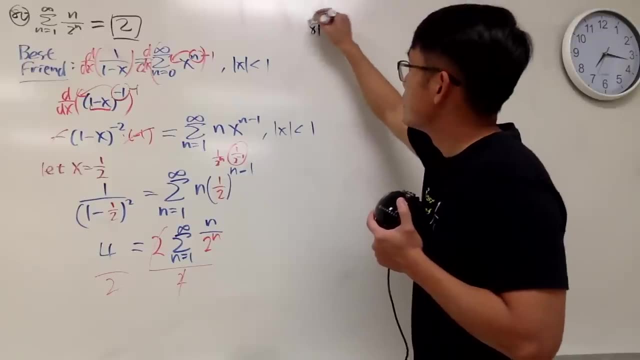 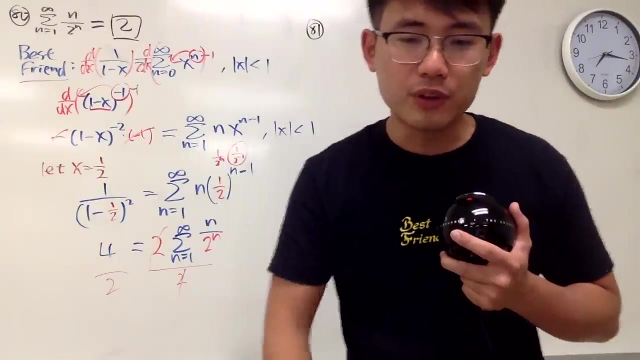 Now here are some of the weirder questions. We'll see number. I wish it was number 90, but we are not there yet. Okay, So we will be asking for what? So that the series will actually converge? 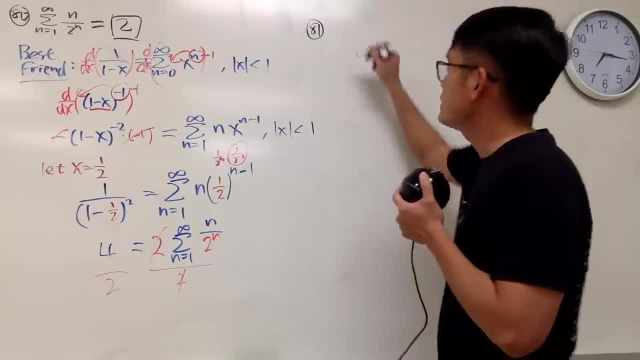 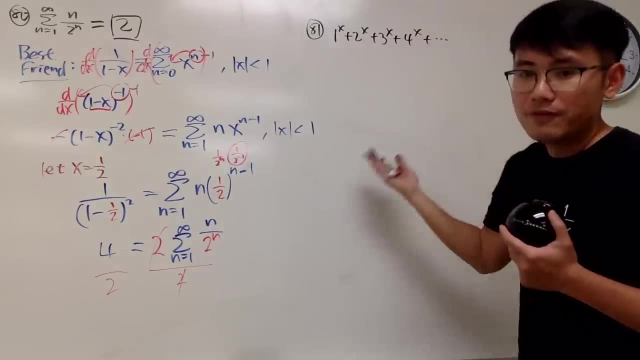 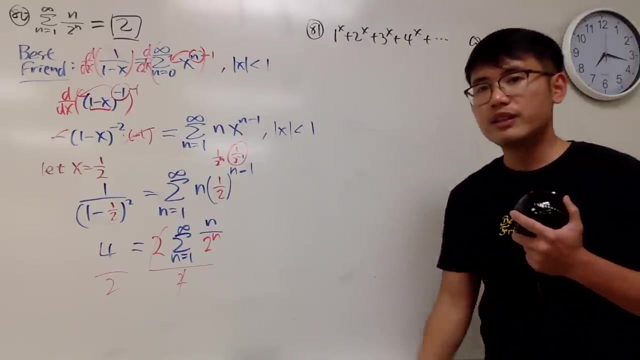 Hmm, For what value will the series 1 to the x plus 2 to the x plus 3 to the x plus 4 to the x plus dot, dot, dot? what value will this converge? So we want to find the condition on the x. 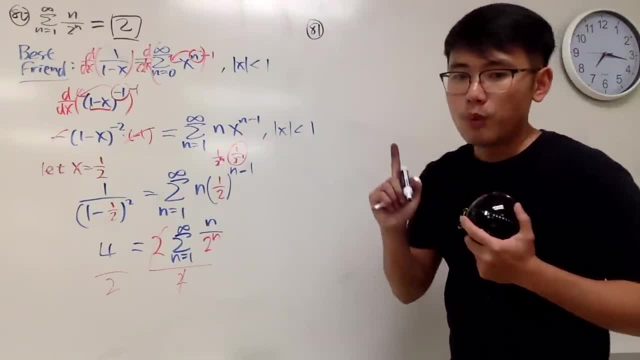 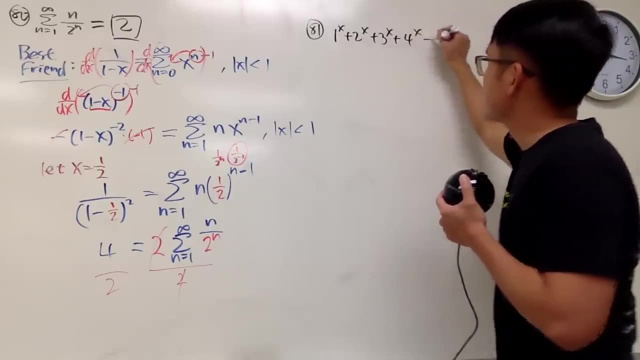 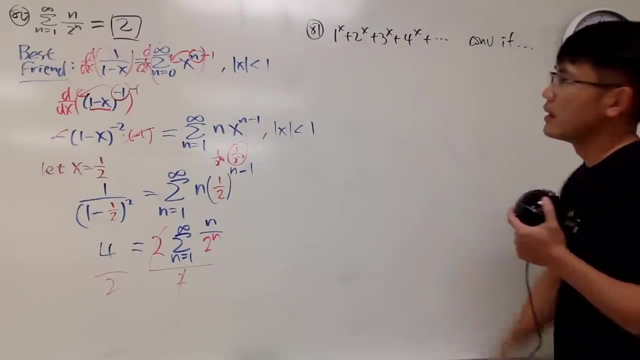 actually converge? Hmm, For what value will the series 1 to the x plus 2, to the x plus 3, to the x plus 4, to the x plus dot dot dot? What value will this converge? So we want to find the condition on the x. Well, if you. 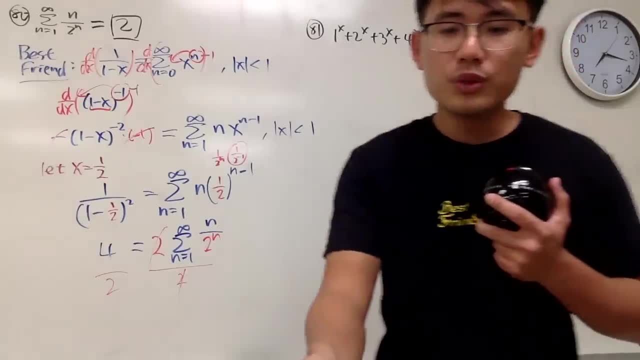 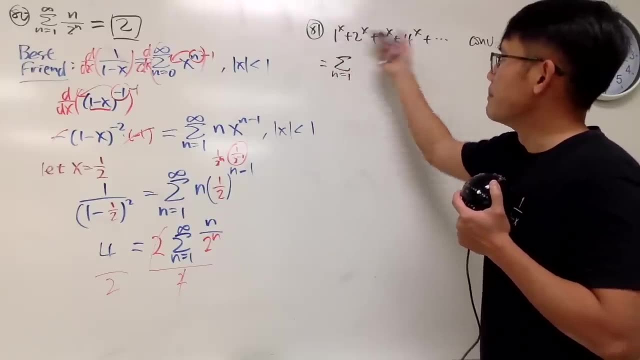 don't like this form too much. you can just put that in the sigma notation. So we will just do that real quick. This is the sum and, as you can see, we have n. start with 1, that's the base, and up to infinity, because of the dot, dot, dot, We have n to the x power. 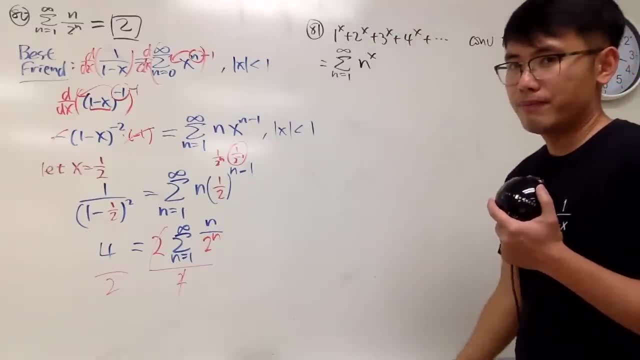 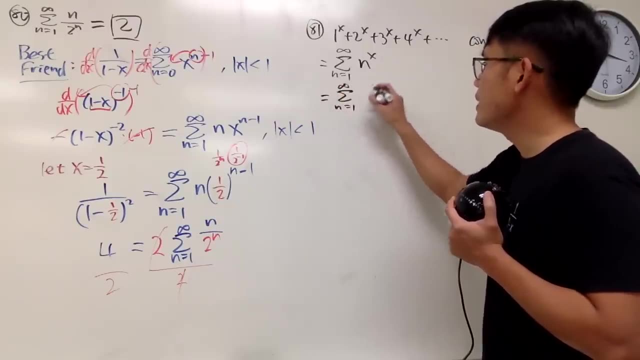 like this, And what does this remind you of? n to the p is power, but that's in the denominator. So do this. This is the same as saying the sum, as n goes from 1 to infinity. 1 over n to the negative x. Right, And now we know. 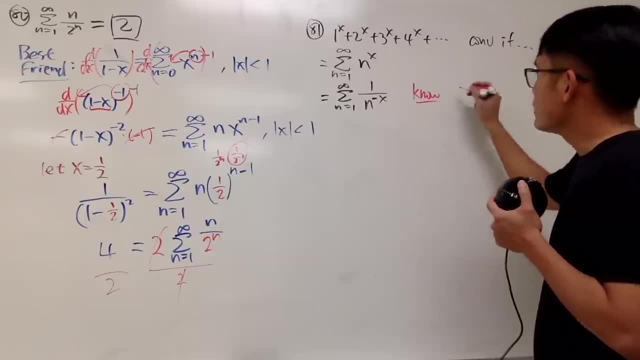 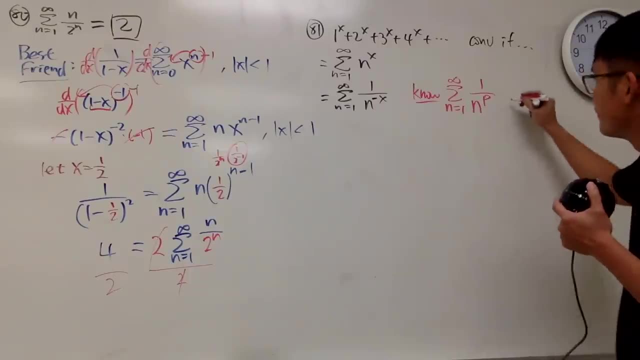 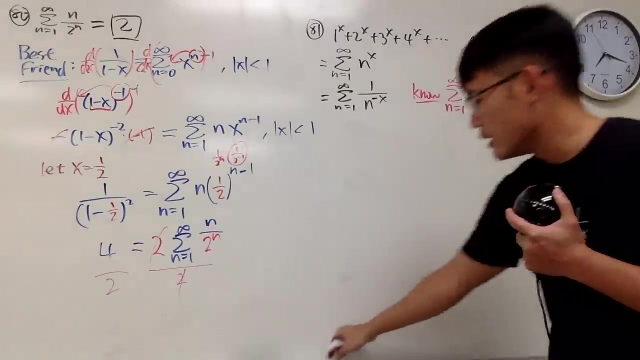 that, thanks to the p series, we know that when we have the sum as n goes from 1 to infinity, 1 over n to the p, this right here converges if p is greater than 1.. What we have to do is look at the power here which is negative, x, and look at the p. We 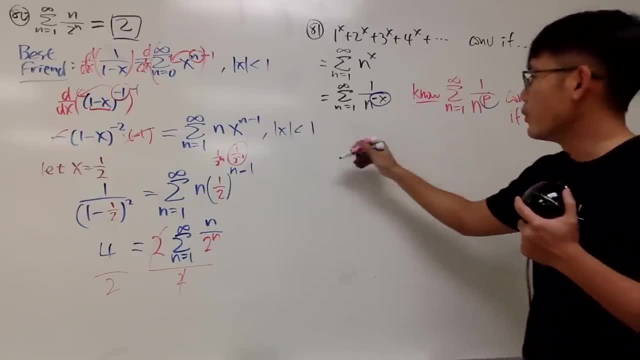 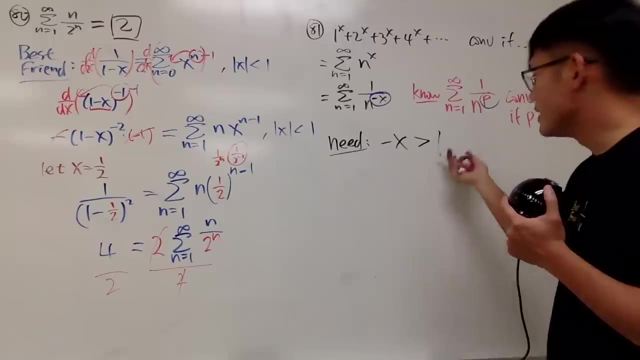 want this right here to be greater than 1.. So we need to have negative x to be greater than 1.. So what does that mean? Of course, divide both sides by negative 1, and this time you have to flip the inequality so we get x is less than 1.. So this is the answer. 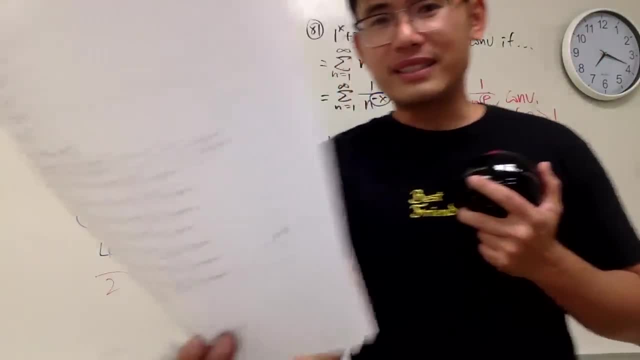 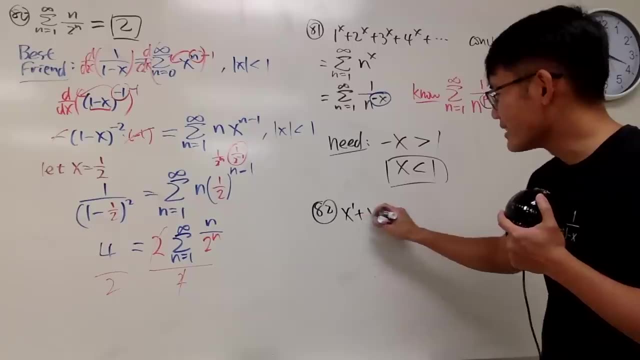 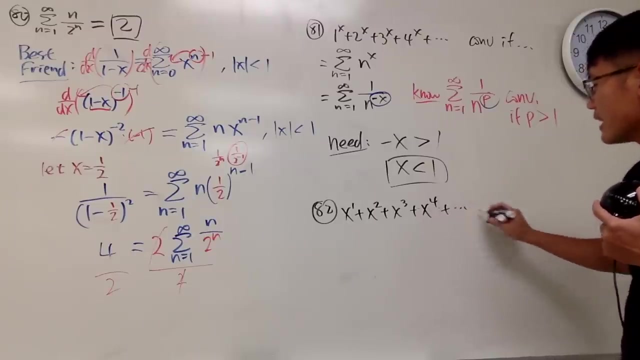 for that. Secondly, for one x, if we switch the place a little bit, let's see 8 to the p2.. Here we have x to the first plus x to the second, plus x to the third, plus dot dot dot. Let's just put on one more term: x to the fourth plus dot dot dot. converge if the 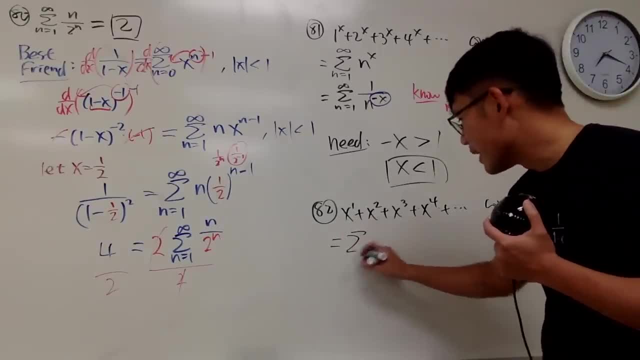 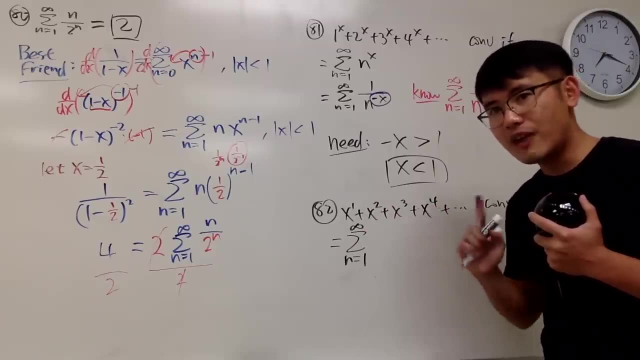 following. Well, this right here it's actually just a sum, as n goes from 1 to infinity, but this time the n is the exponent, So we have the x for the base right here, n raised to the nth power, and this is the what. 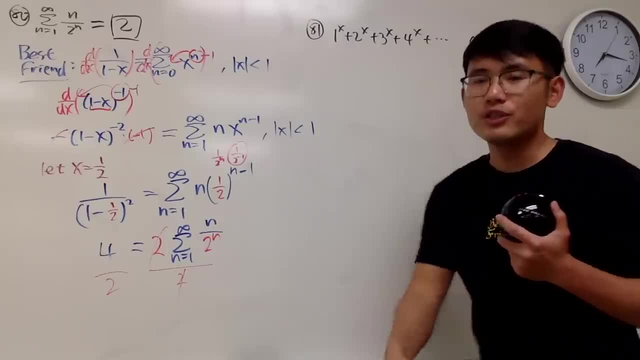 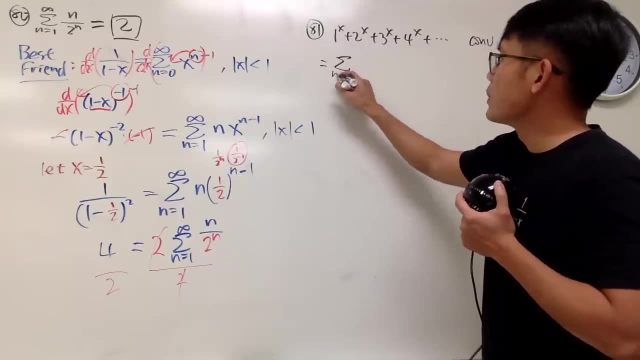 Well, if you don't like this form too much, you can just put that in the sigma notation. So we will just do that real quick. This is the sum And, as you can see, we have n start with 1, that's the base, and up to infinity because of the dot, dot, dot. 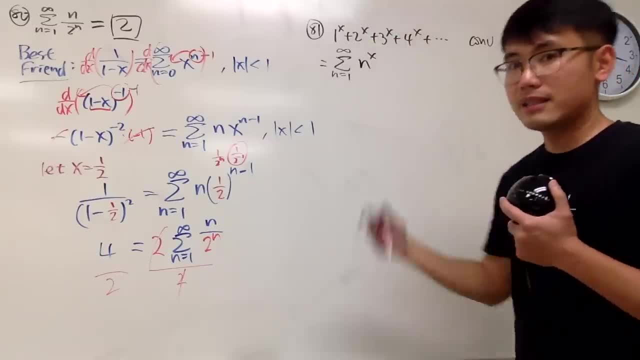 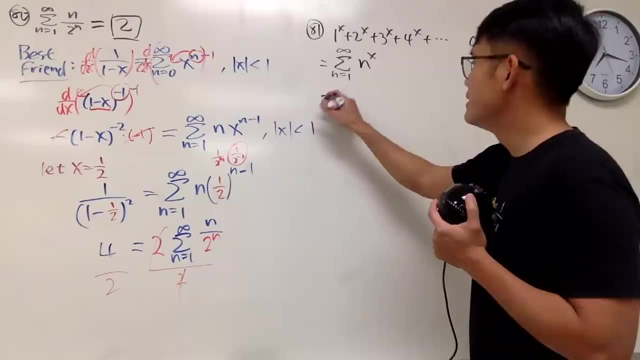 We have n to the x power like this. And what does this remind you of? n to the p's power, but that's in the denominator. So do this. This is the same as saying the sum, as n goes from 1 to infinity, 1 over n to the negative x. 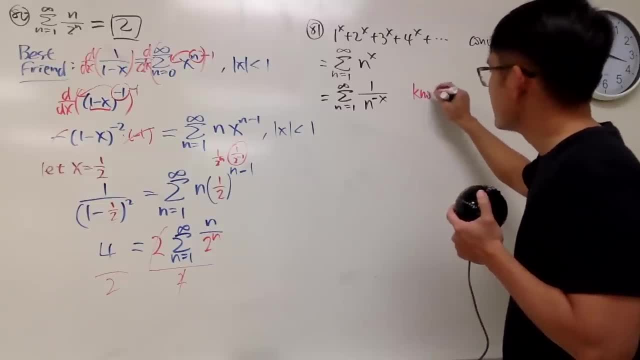 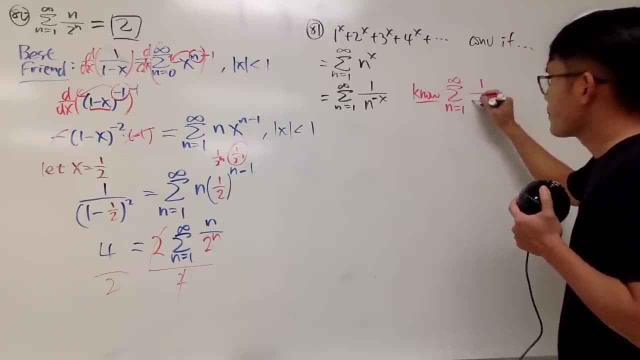 Right. And now we know that, thanks to the p series, we know that when we have the sum as n goes from 1 to infinity, 1 over n to the p, this right here converges if p is greater than 1.. 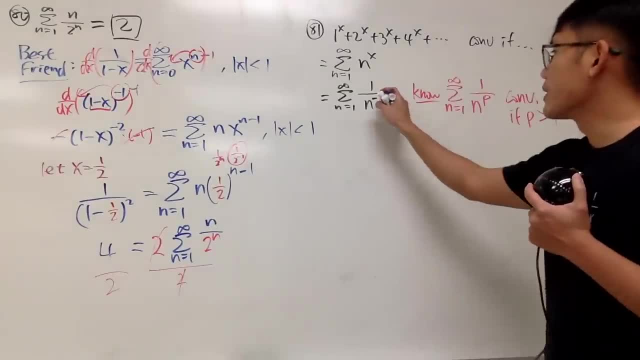 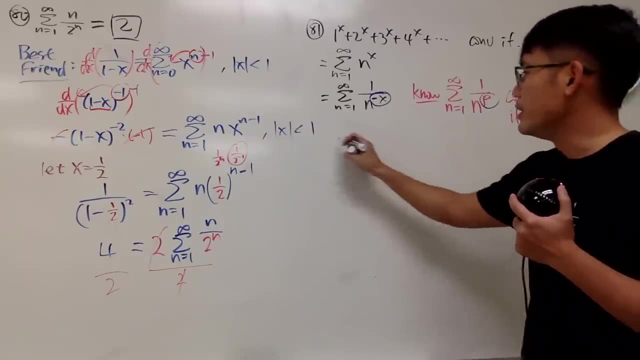 So now all we have to do is look at the power here, which is negative x, and look at the p. We want this right here to be greater than 1.. So we need to have negative x to be greater than 1.. 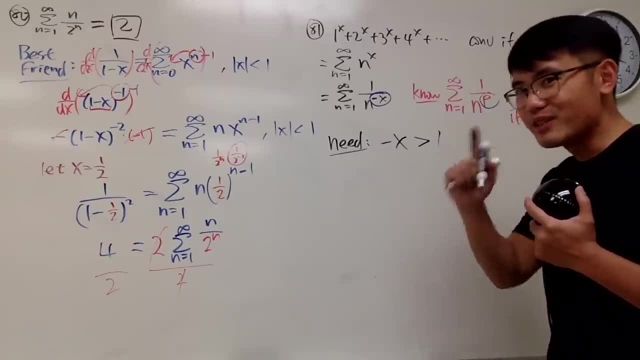 So what does that mean? Of course, divide both sides by negative x. So what does that mean? Of course, divide both sides by negative 1, and this time you have to flip the inequality so we get x is less than 1.. 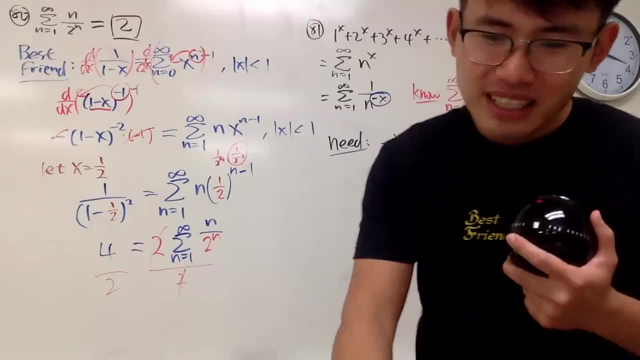 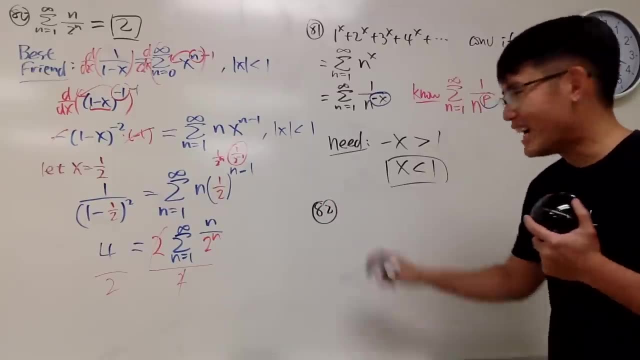 So this is the answer for that. Secondly, for one x, if we switch the place a little bit, let's see 82. Here we have x to the first, plus x to the second, plus x to the third, plus dot dot dot. 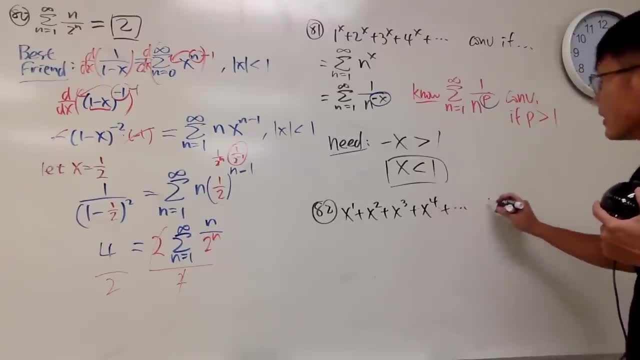 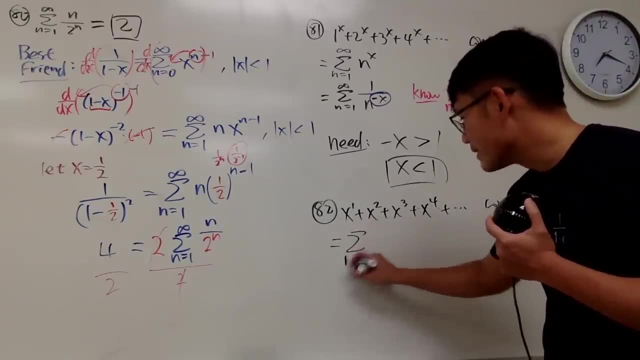 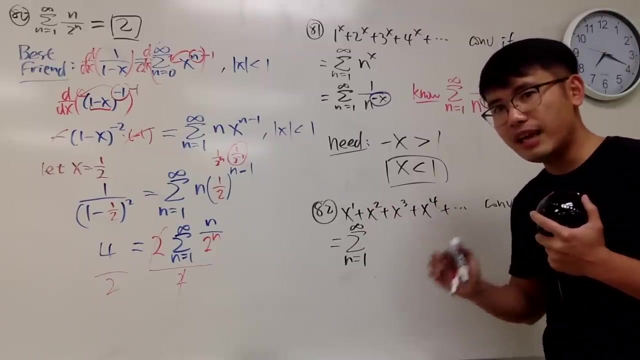 Let's just put on one more term: x to the fourth plus dot, dot, dot converge if the following: Well, this, right here, It's actually just the sum, as n goes from 1 to infinity, but this time the n is the exponent, so we have the x for the base, right here. 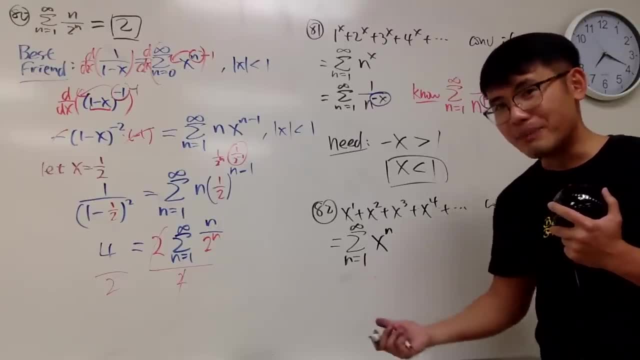 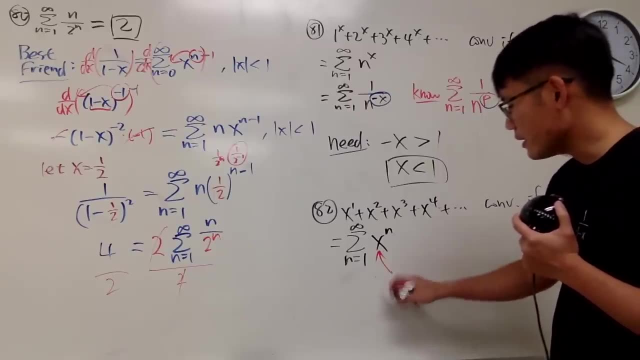 n raised to the nth power, and this is the what The best friend, So this right here, we'll just say we need the r is just x and, as we all know, take it up for you to be less than 1.. 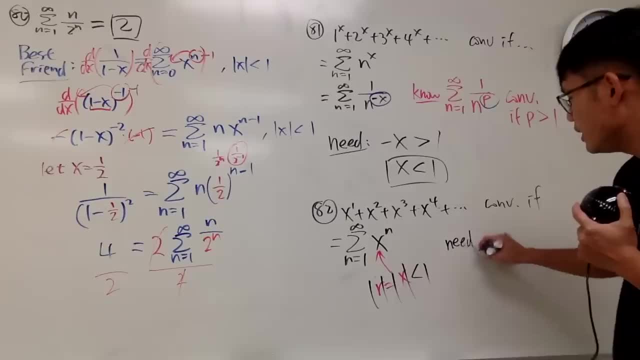 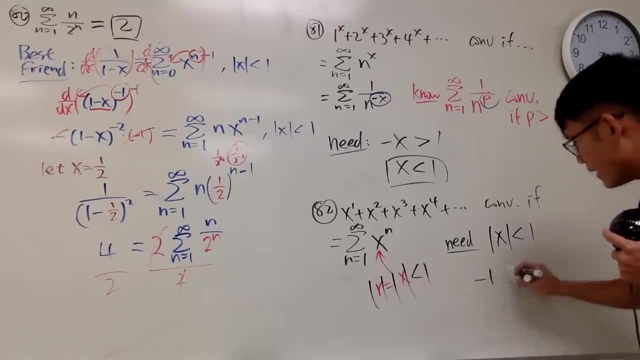 That's pretty much the idea. So I'll just tell you: We need the absolute value of x to be less than 1, and you can break this inequality down as negative 1, x is in between negative 1 and 1, so one way or the other for it. 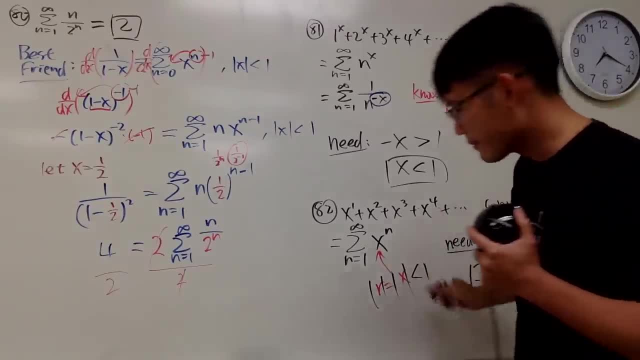 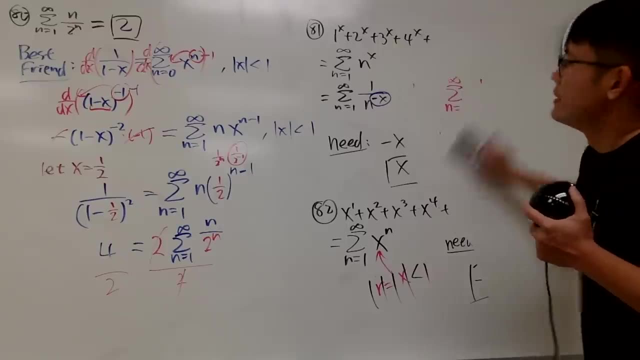 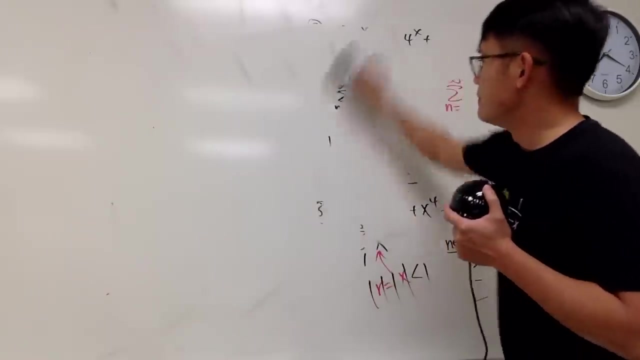 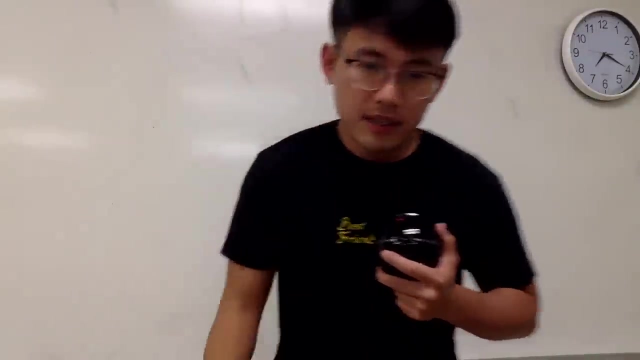 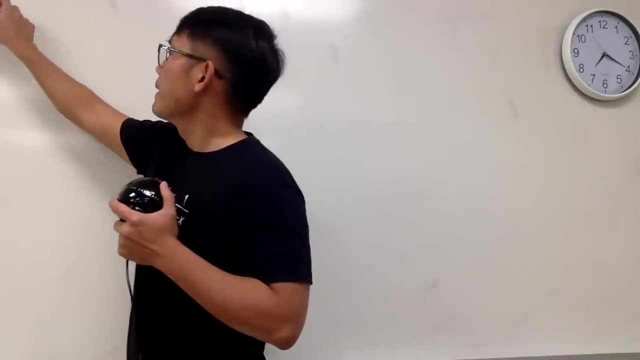 And we do not include an endpoint for the best friend. okay, So that's it for that. Very, very nice right? So, man, that took me some time for the number 80, so we will see. Okay, now for what value of the series, let me see. let me write down 83. 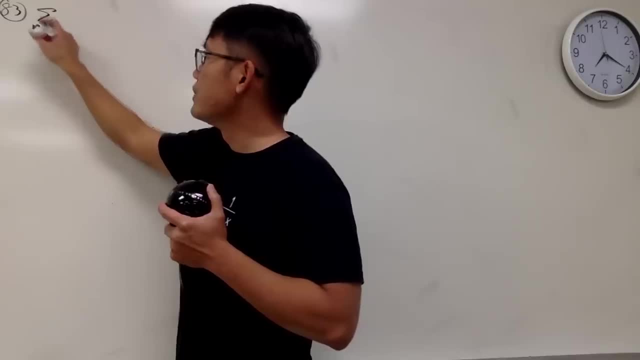 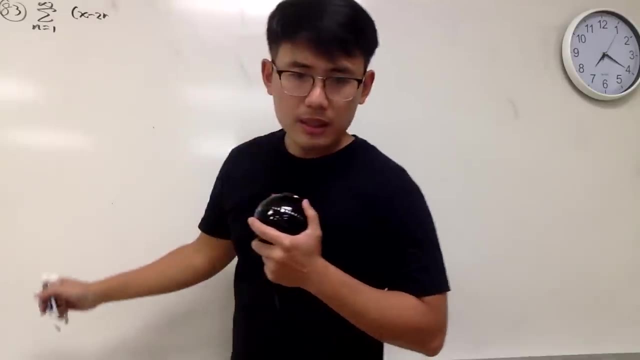 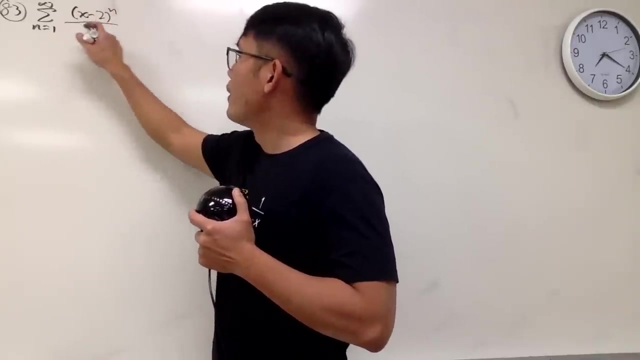 Again, we are looking for the x so that it converges. okay, the series converges. We have this right here and we have x minus 2 and raised to the nth power. So we have x minus 2 over n to the nth power, like that. 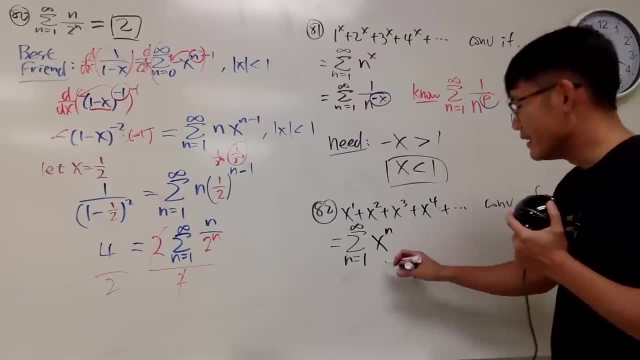 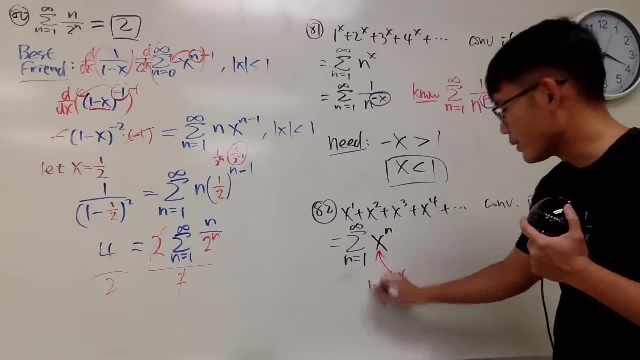 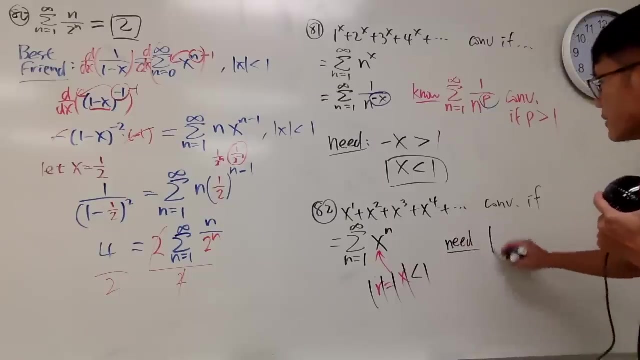 The best friend. So this, right here, we'll just say we need the r is just x and, as we all know, take the absolute value to be less than 1.. That's pretty much the idea. So I'll just tell you: we need the absolute value of x to be less than 1, and you can break. 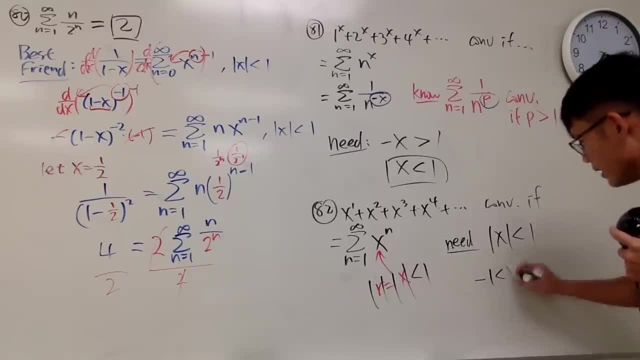 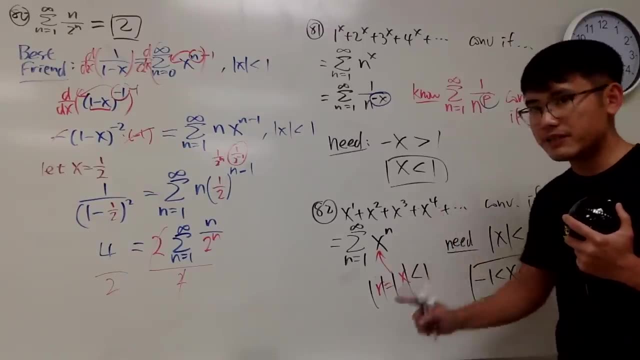 this inequality down as negative 1,. x is in between negative 1 and 1, so one way or the other for it, And we do not include an endpoint. Well, this is just for the n Boolean quotient we just used here, So we're just going to. 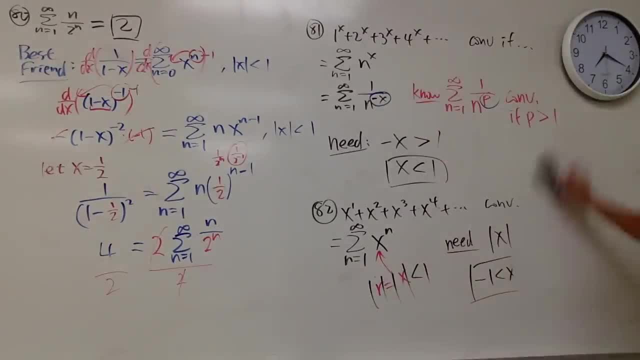 take x to the left minus 1, and 0 to the right minus 1,, because if the left is the absolute value, then the value of x to the right is 1.. So the other way around. we can just say: 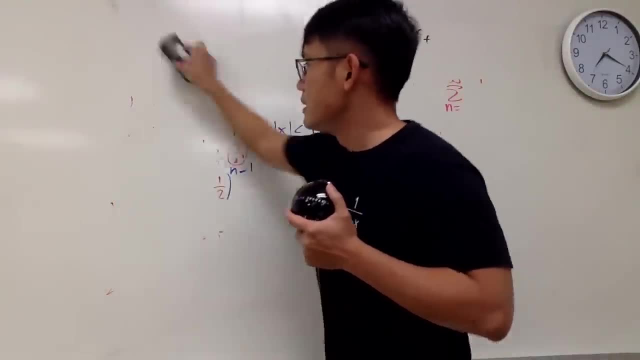 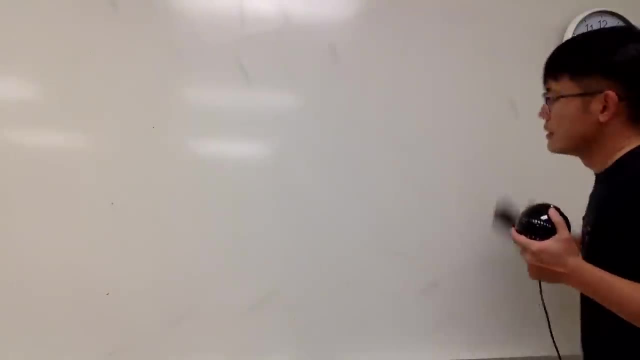 this is the x to the left. We're going to use the r equals 1 to the right And this is the value of x to the left. And then I just want to make sure that you all know the past number. So this is the nth power of x to the left. We're going to take the absolute. value of x to the right, and then we're going to take the maximum value of x to the left, And if the aspect ratio is negative, 1, then the value of x to the left is 0.. So it's all for the nth power. So we'll just say: what is this? 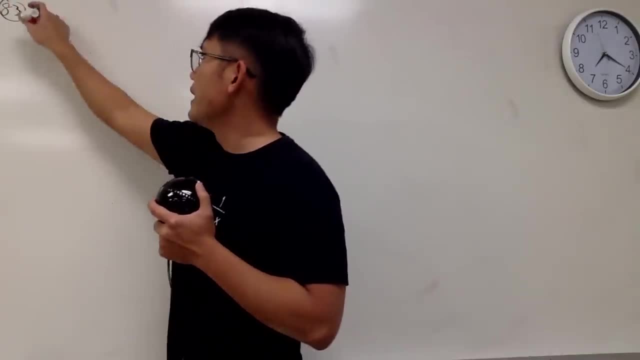 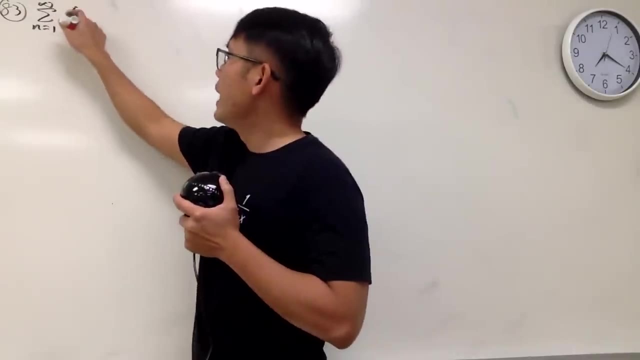 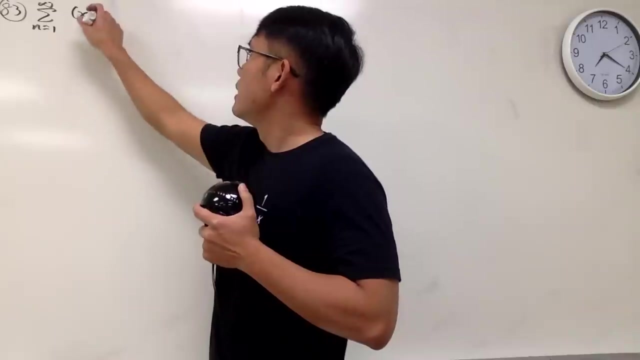 83. Again, we are looking for the x so that it converges. okay, the series converges. We have this right here and we have x minus 2 and raised to the nth power over n to the nth power, like that. 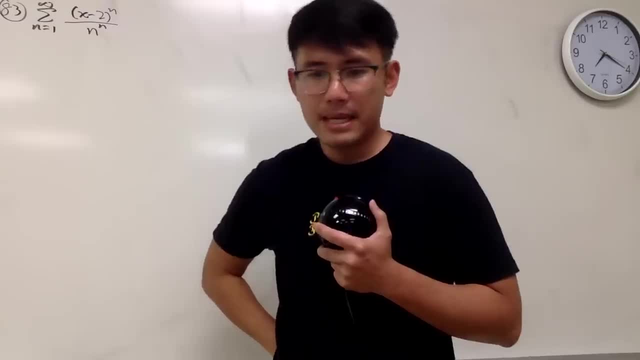 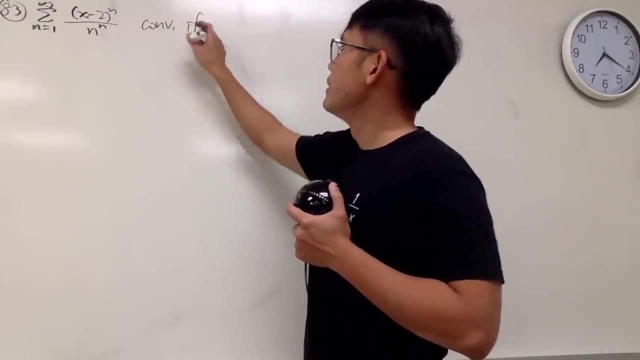 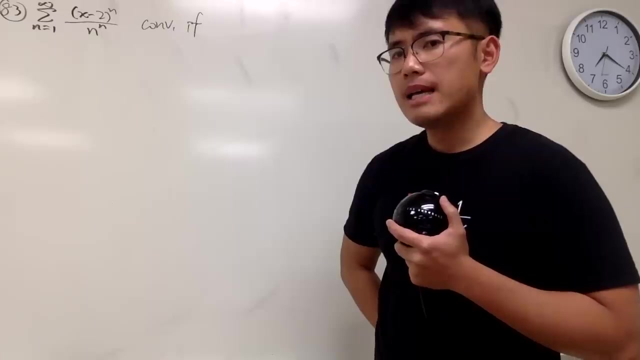 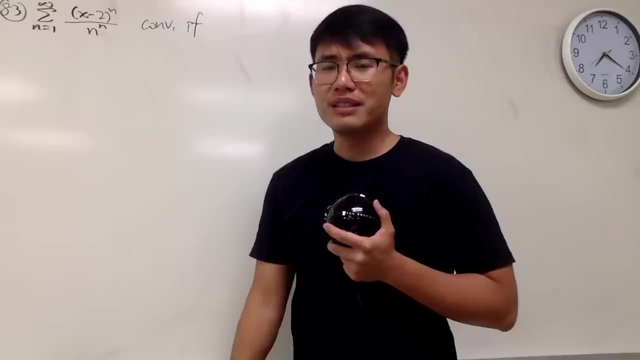 Hmm, You can try to. well, I'll just say well, I'll just say converge, if what happened right. Maybe we can do the root test, because you see, when we have the n in the exponents, to do root test is pretty useful. You can also do the ratio test. 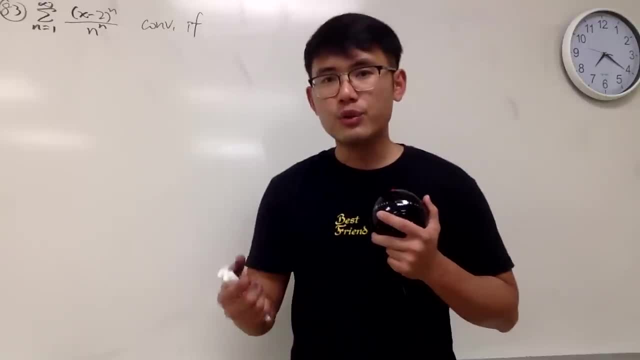 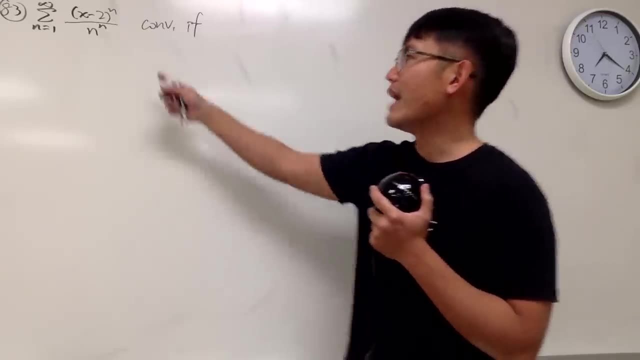 Let me tell you, this kind of question is pretty, pretty much for asking you for the radius of convergence for power series, And usually the ratio test will be the way to go. However, here we have n and n in the exponents, so a better choice is the root test. 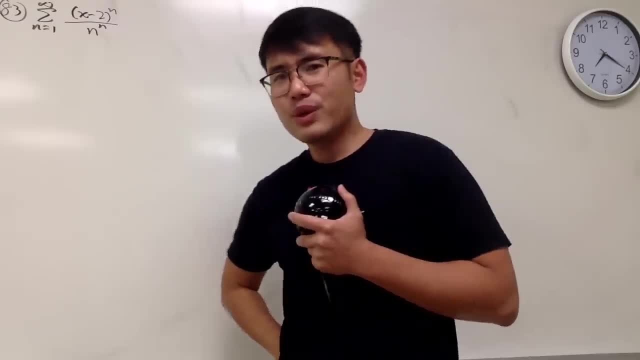 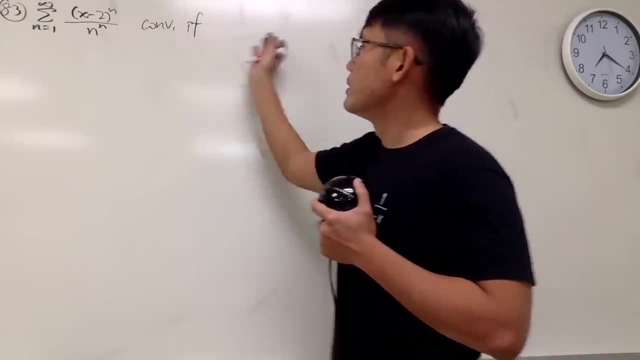 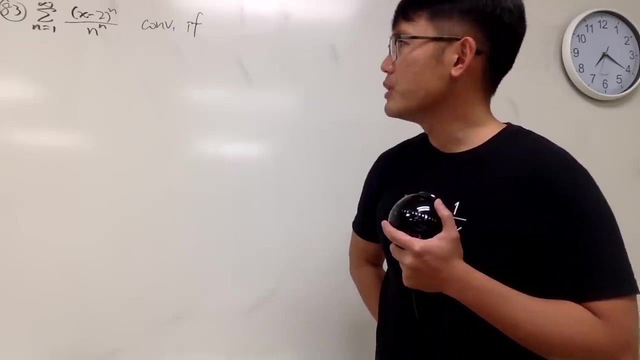 Hmm, You can try to. well, I'll just say well, I'll just say converge. if what happened right, Maybe we can do the root test, Because, you see, when we have the nth power, we can do the root test. 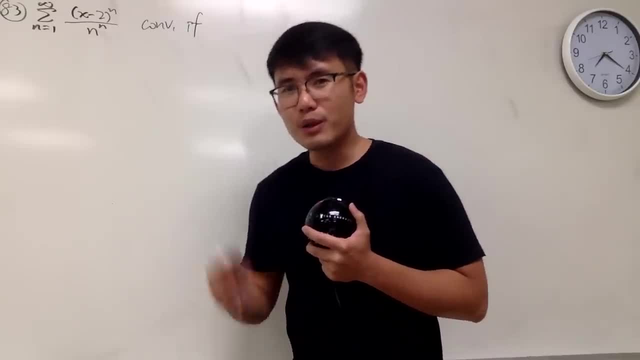 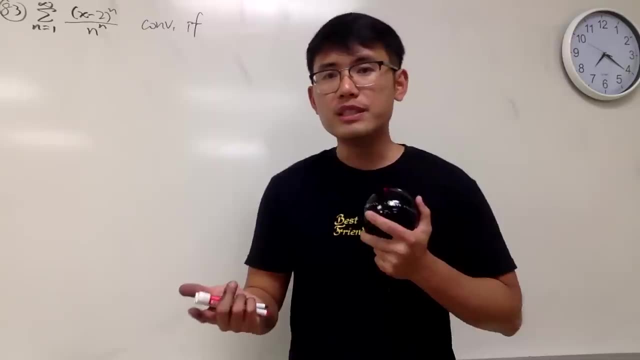 And in the exponents, the root test is pretty useful. You can also do the ratio test, Let me tell you. this kind of question is pretty much asking you for the radius of convergence for power series, And usually the ratio test will be the way to go. 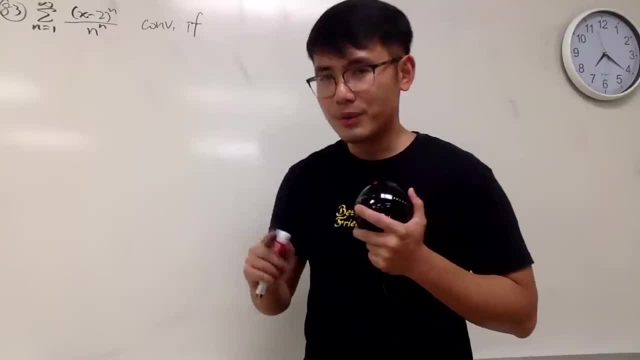 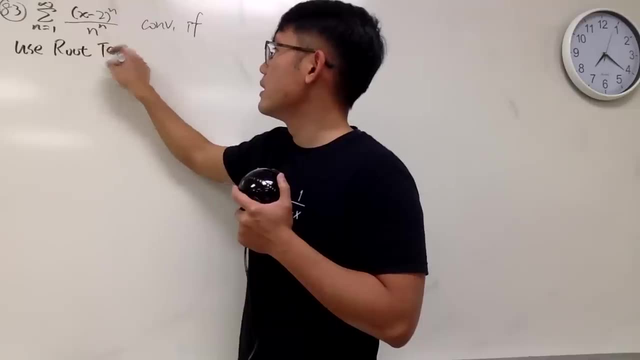 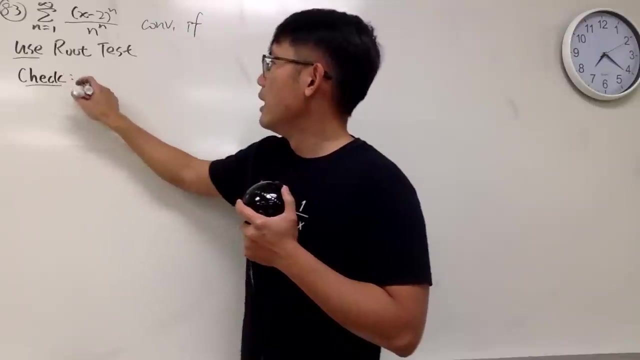 However, here we have n and n in the exponents, so a better choice is the root test. So I'll just tell you guys, we'll use the root test And the idea is that I will just check As n goes to infinity. and let's just take a look of this real quick. 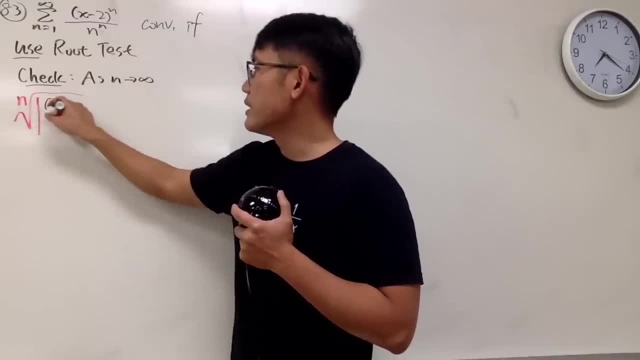 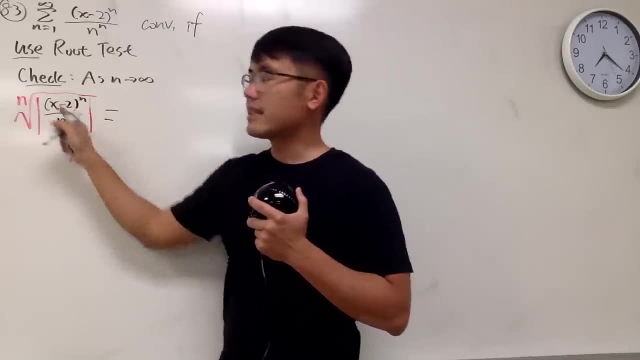 So the nth root absolute value and then the input is x minus 2, n over n to the n, like this: Okay, This and that you guys know the deal. So we just have x minus 2 over n, like this: 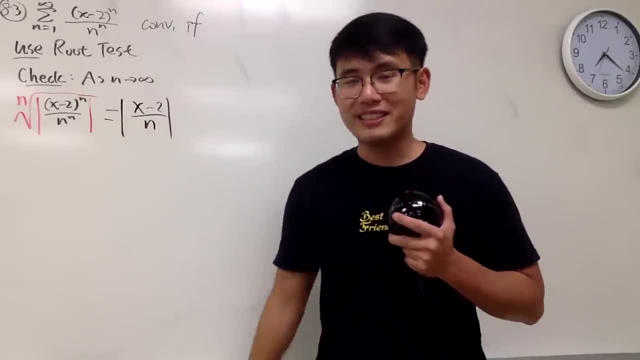 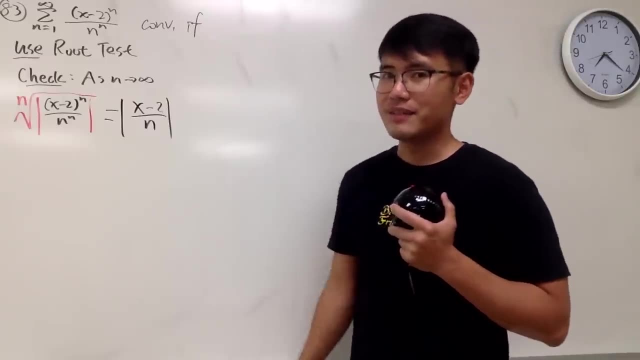 And you have to maintain the absolute value because you don't know what x is. x can be negative, it can be positive. I don't know, So t it like that, but we know for sure n is positive, so we know this right here is actually equal to: 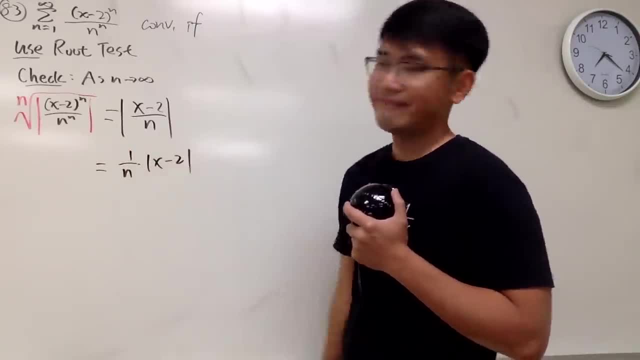 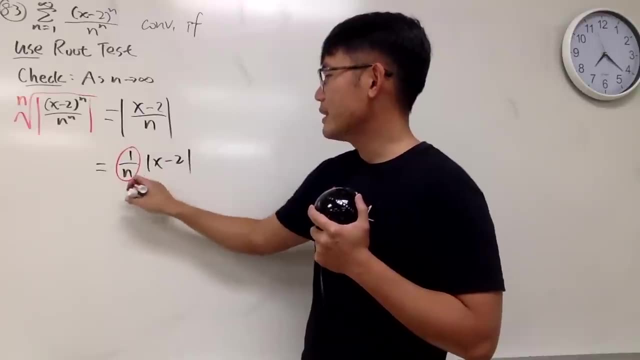 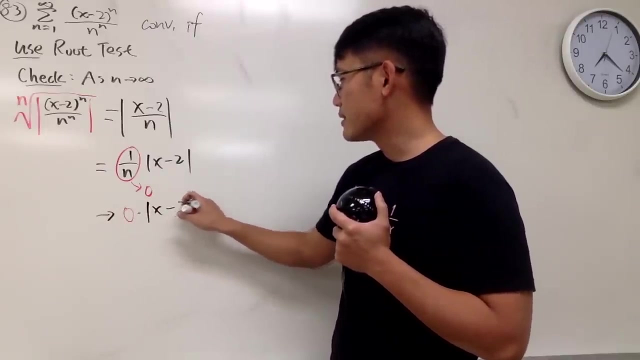 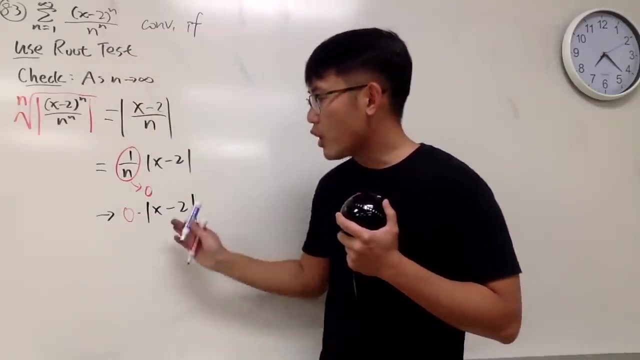 1 over n times absolute value of x minus 2, like this: now, as x is approaching infinity, this right here it's approaching 0. so in another word, we are just getting 0 times absolute value of x minus 2, like this. now, remember when we are using the ratio test for the root test, your goal is to 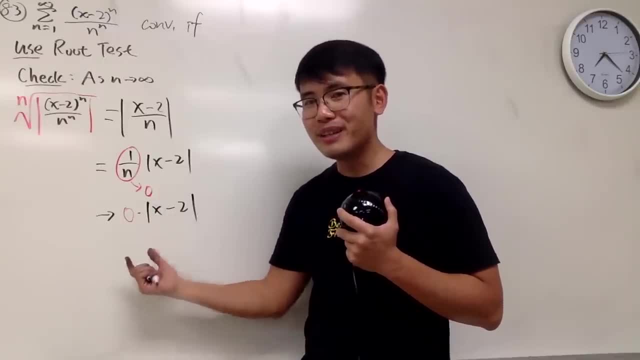 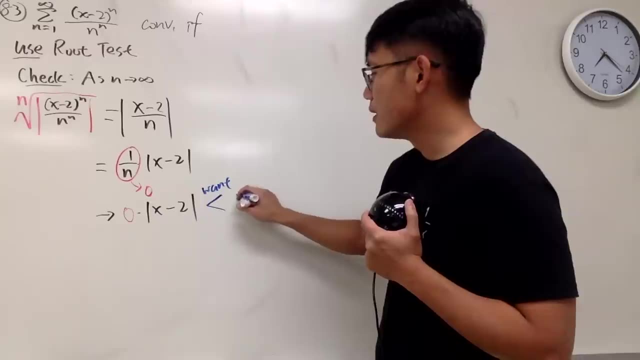 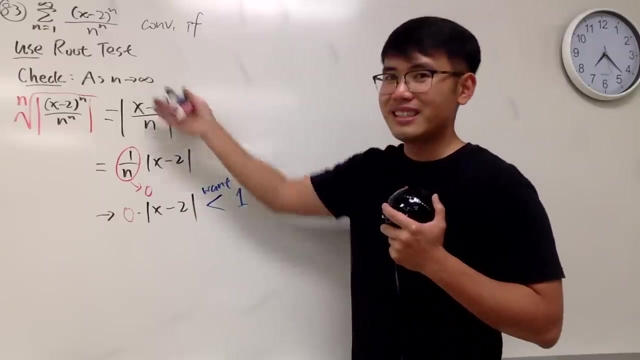 make sure that your limit in the end turns out to be less than 1, so it converges, right. well, how can we make this right here? right, this is what we want down. how can we make this to be less than one? technically, i should have set up right here, but you, you do have to take the limit. 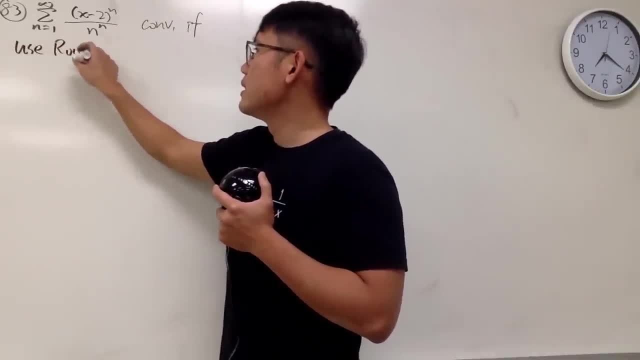 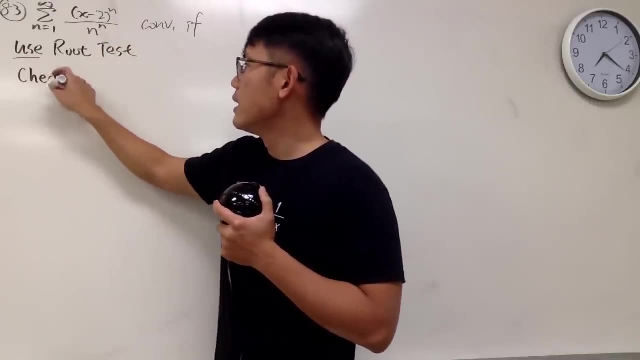 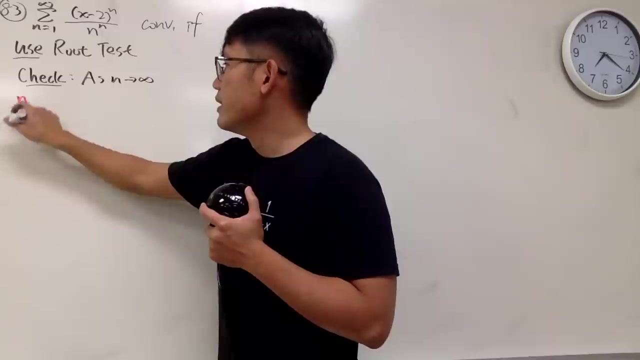 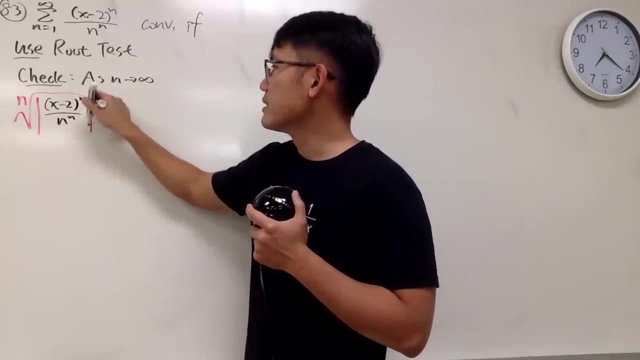 So I'll just tell you guys, we'll use the root test And the idea is that I will just check s n goes to infinity, And let's just take a look after this real quick. So we have the nth root absolute value and then the input is x minus 2 n over n to the n, like this: 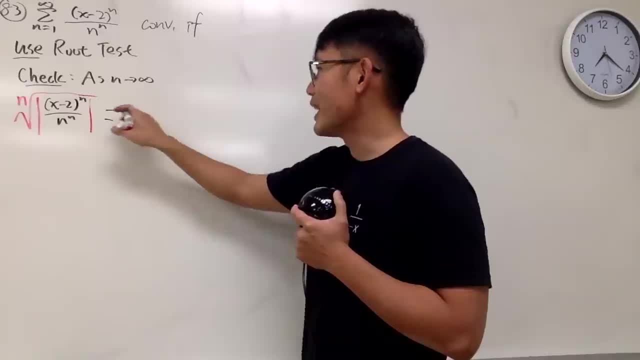 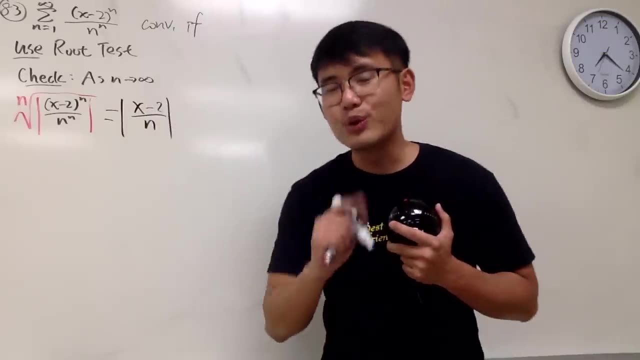 Okay, this and that you guys know the deal. so we just have x minus 2 over n, like this, And you have to maintain the absolute value, because you don't know what x is. x can be negative, it can be positive, I don't know, so keep it like that. 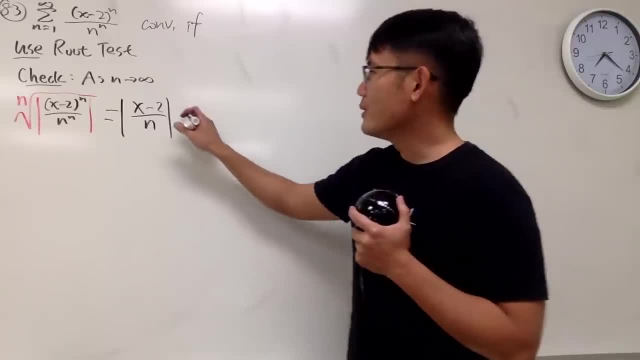 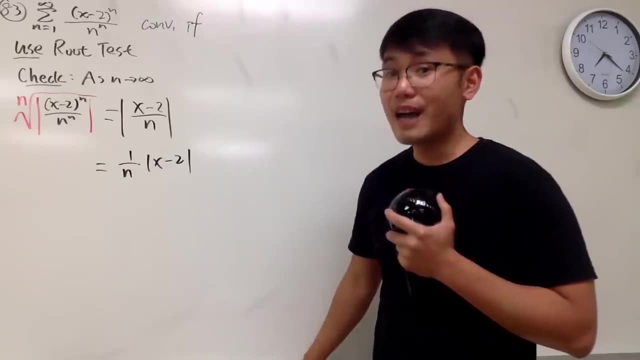 But we know for sure n is positive, So we know this right here is actually equal to 1 over 2.. 1 over n times absolute value of x minus 2, like this: Now, as x is approaching infinity, this right here it's approaching 0.. 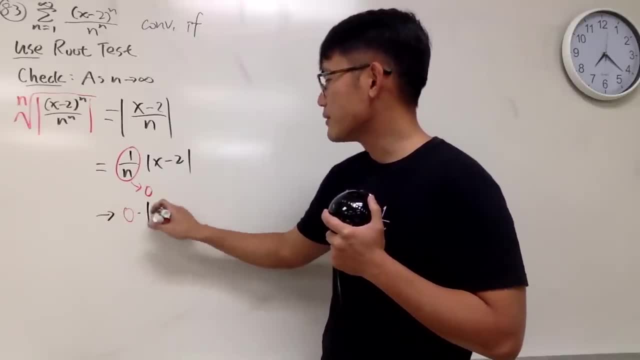 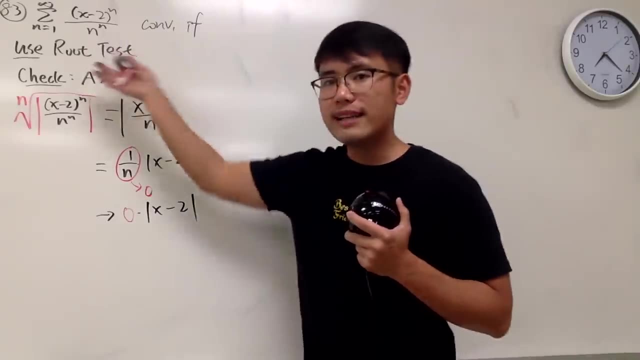 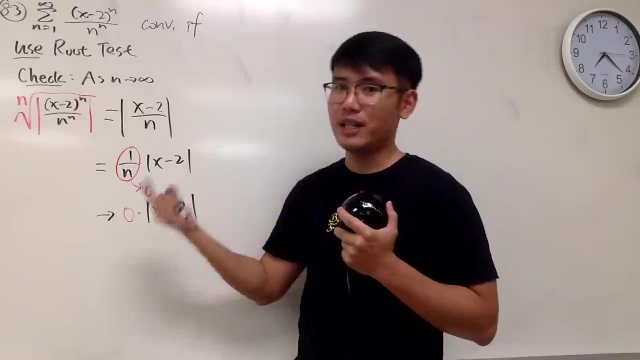 So, in another word, we are just getting 0 times absolute value of x minus 2, like this. Now remember when we are using the ratio test for the root test. your goal is to make sure that your limit in the end turns out to be less than 1, so it converges. 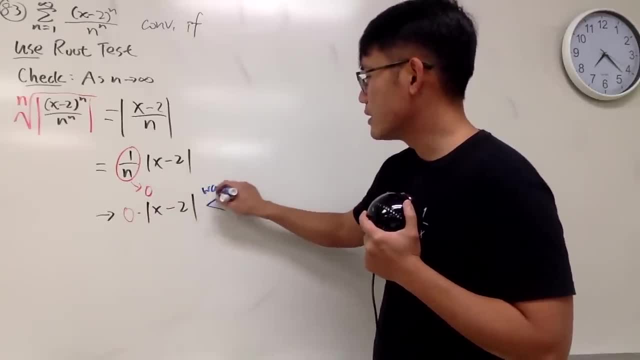 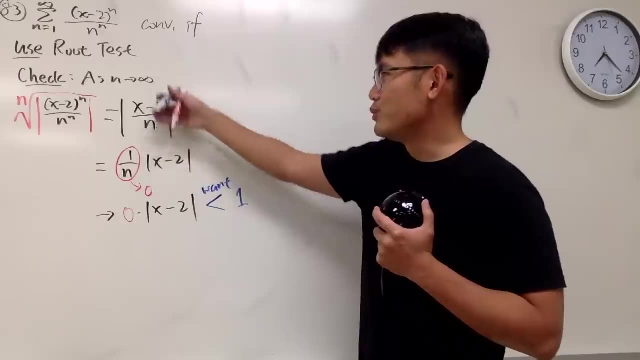 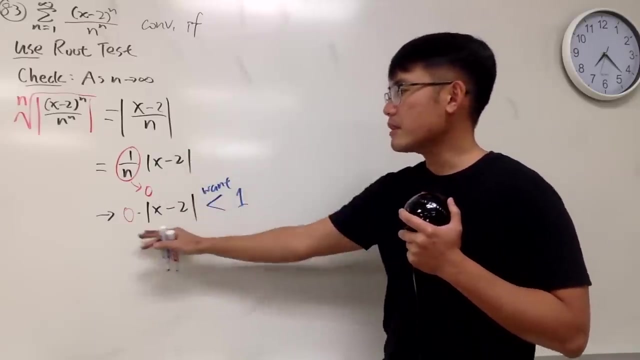 Well, how can we make this right here? this is what we want now. how can we make this to be less than 1?? Technically, I should have said that right here, but you do have to take the limit first. The deal is that once you take the limits right here, n approaching infinity, this is just 0,. 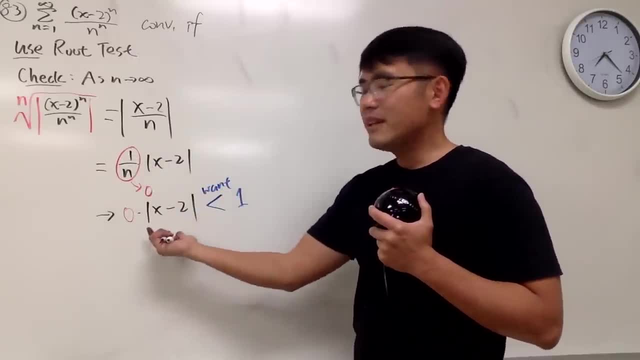 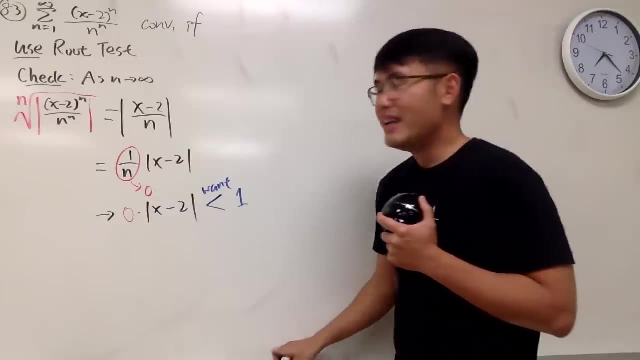 and remember, x is just some finite number. Can you give me any number? in putting here times 0?, That will also be less than 1, right, Of course? this is the idea, So the truth is, I will actually rephrase it. 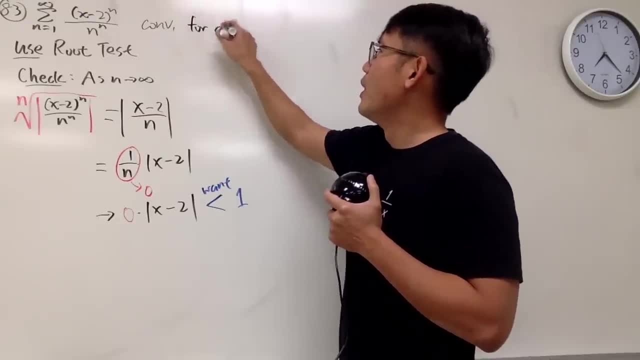 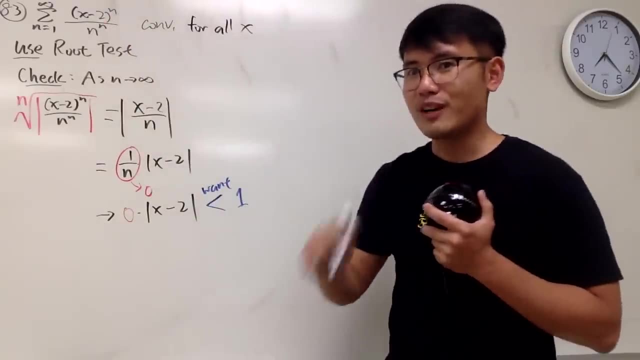 This right here actually converges for all x. You can give me any x value, put it here. that series will converge, guaranteed, And it has to be like 5,, 7, or 28, or 2019, or something like that. 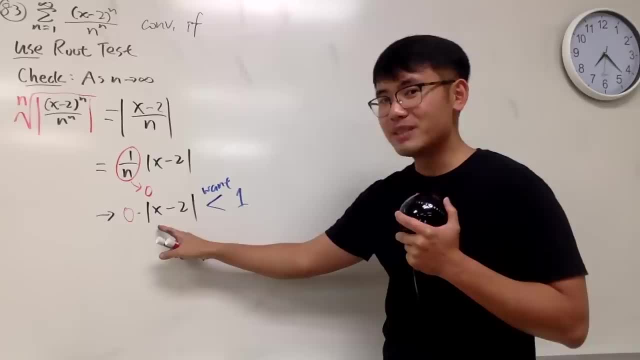 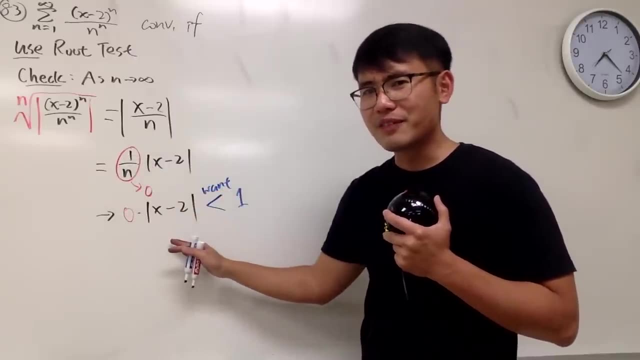 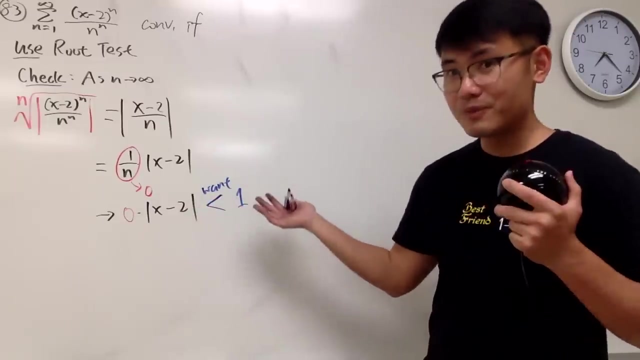 first, the deal is that once you take the limits right here, right, okay, n approaching infinity, this is just 0. and remember, x is just some finite number. can you give me any number? in putting here times 0, that will also be less than 1, right, of course. 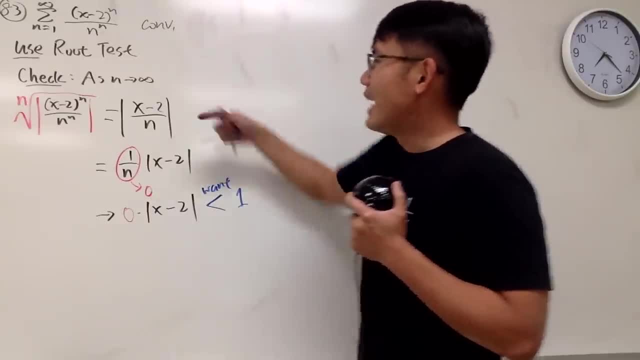 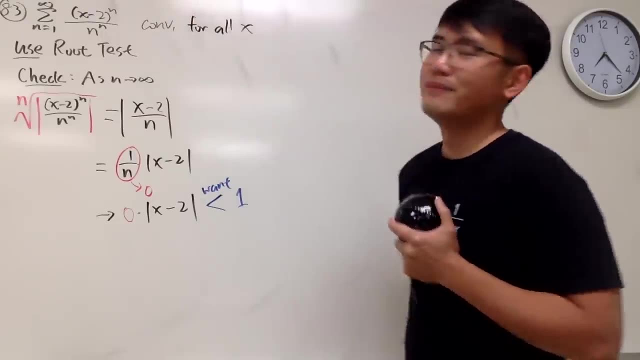 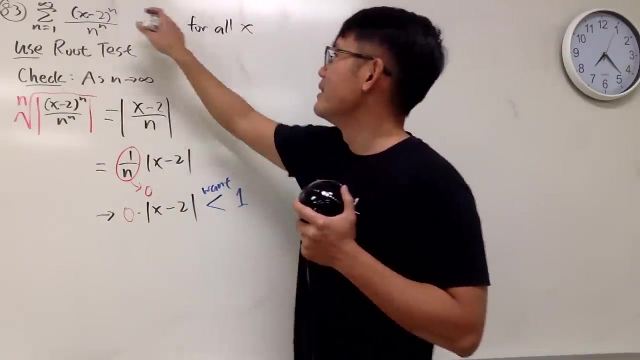 this is the idea. so the truth is- i will actually rephrase it this right here: actually: converges for all x. you can give me any x value, put it here. that series will converge, guaranteed, and it has to be like 5, 7 or 28 or 2019 or something like that. you cannot say put. 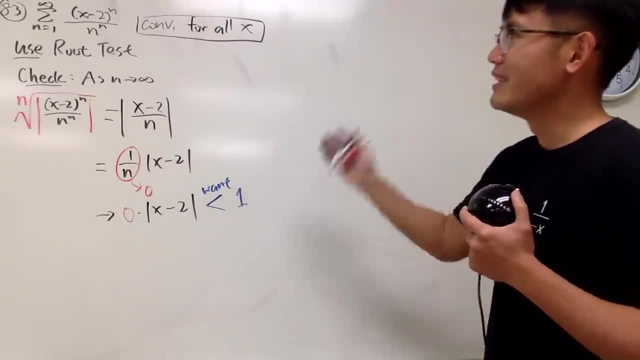 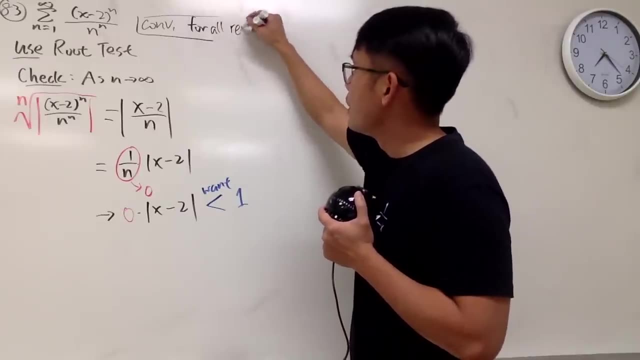 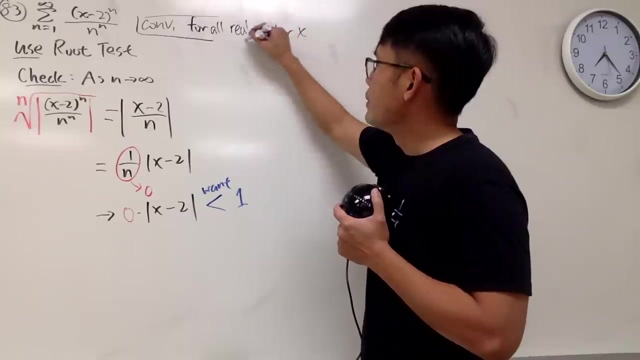 infinity there. infinity is not a number, but for all real number of x, like that, for all x. i'll just say for all, for all real x, for all real number x. or you can also put on negative infinity to positive infinity. in that case you are telling the 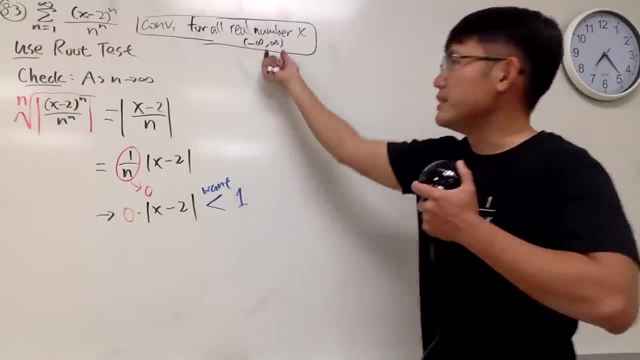 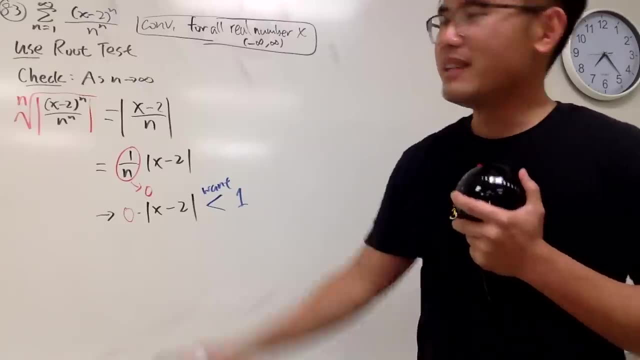 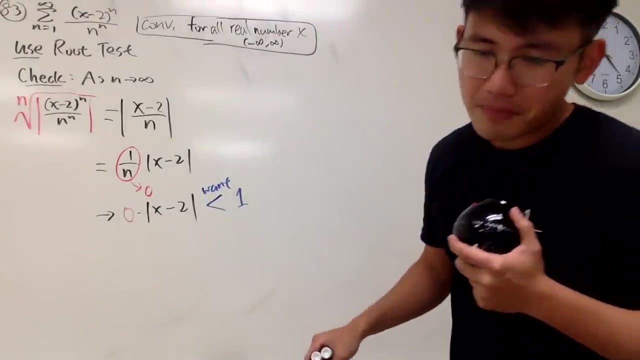 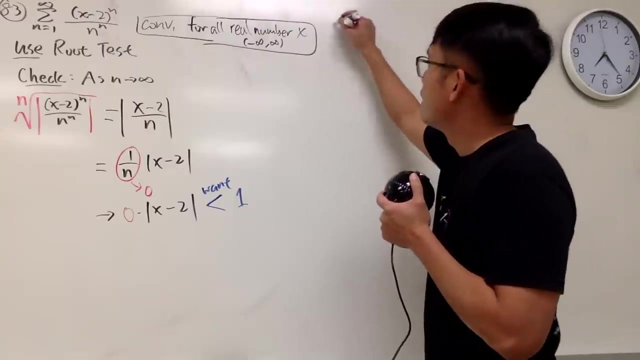 um radius of convergence, or technically this is interval convergence- to have the half series work. that's not quite the power. well, that's a power series, but the other ones that i'm demonstrating not so much. you'll see all right now, number 84, uh, we are going to do the same thing. 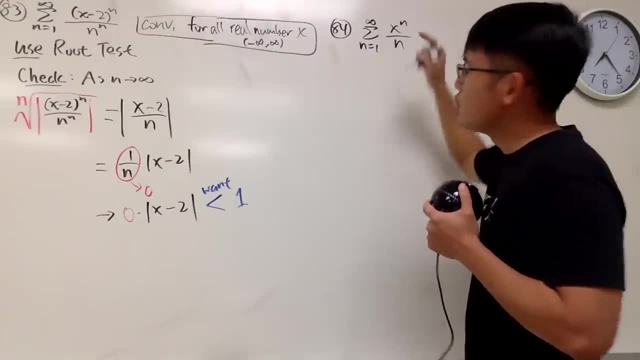 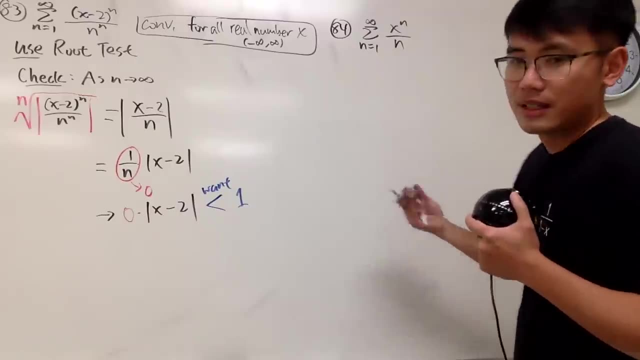 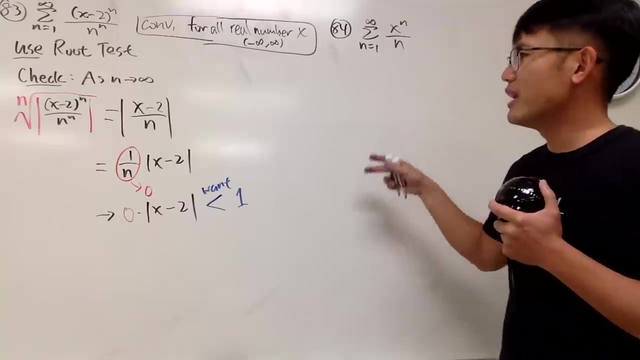 some goes from 1 to infinity, x to the n over just an n, all right. and then, yeah, i want to see when does this converge? well, if you do the root test, i think it's still okay, because we know how to handle that. but now let me show you guys how you use the ratio test. 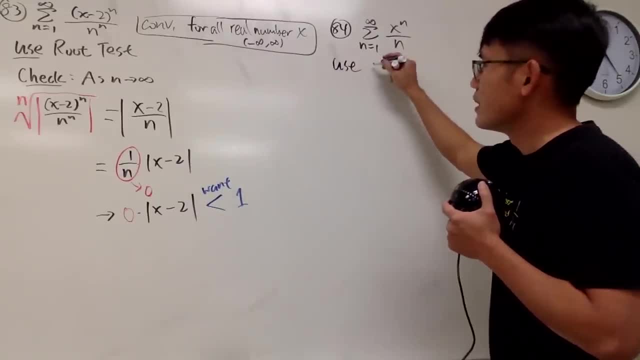 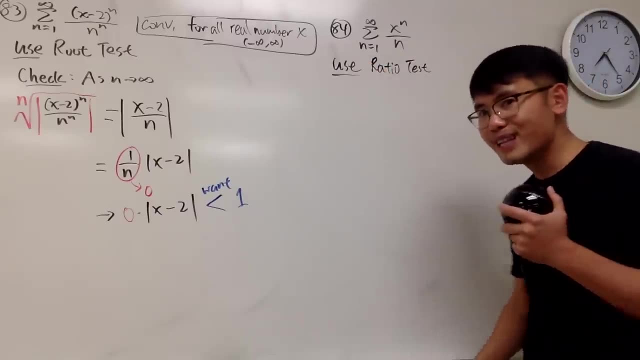 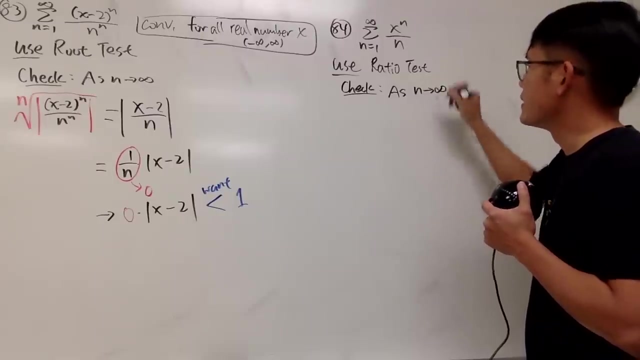 and earlier you could have used the ratio test as well, right? so let me just say: use the ratio test. now here's the po. check the limit as x. so as n goes to infinity ratio test in action. here we have x- i don't know what it is yet- and then you raise that. 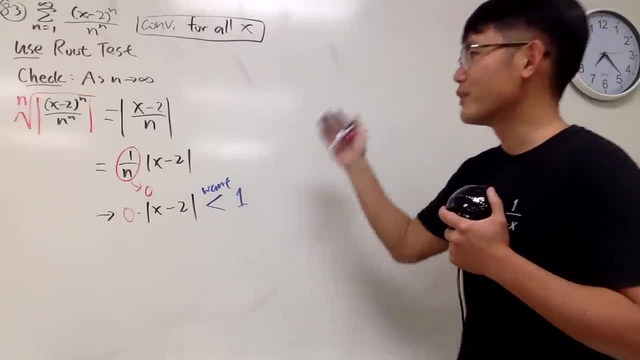 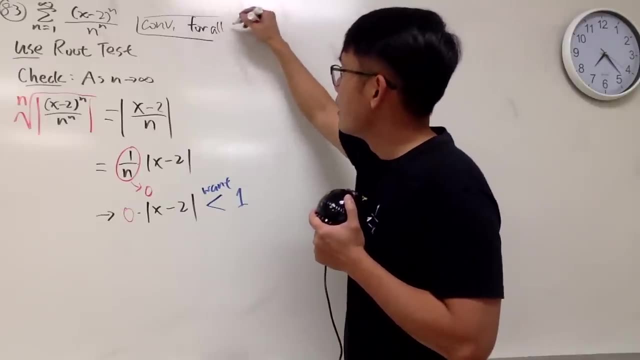 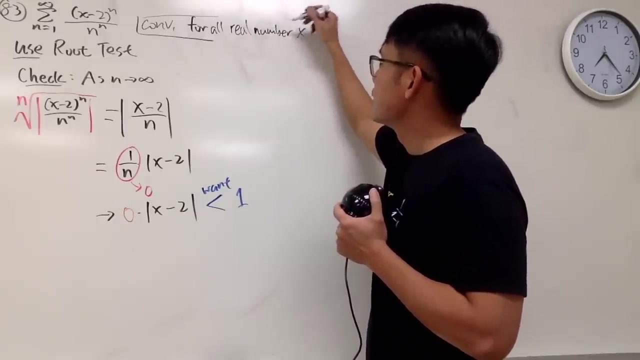 You cannot say put infinity there. infinity is not a number, but for all real number of x, like that, for all x, I'll just say for all real x, for all real number x. Or you can also put down negative infinity to positive infinity. 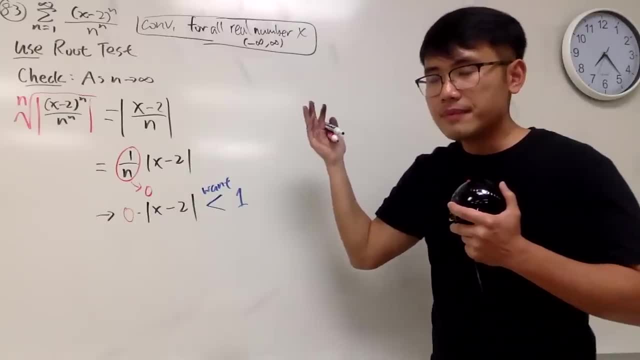 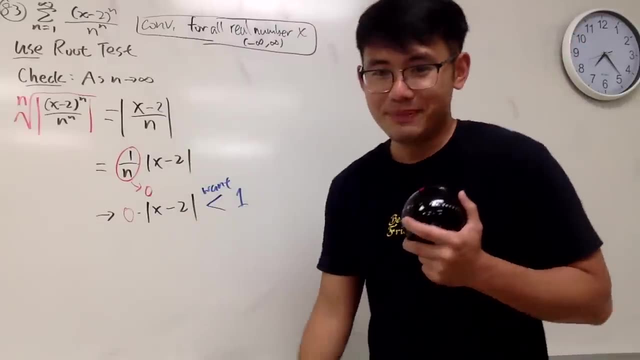 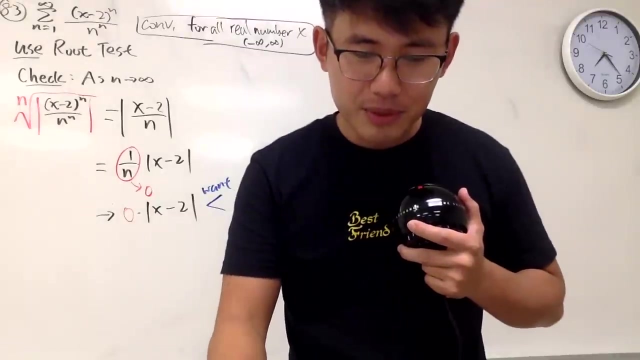 In that case you are telling the radius of convergence, or technically this is interval convergence, to have that series work. That's not quite the power series. Well, that's a power series, but the other ones that I'm demonstrating not so much. 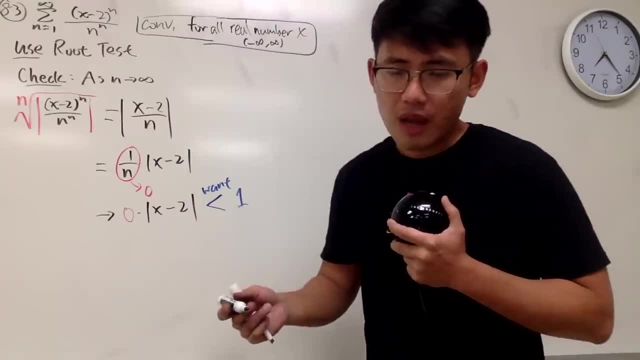 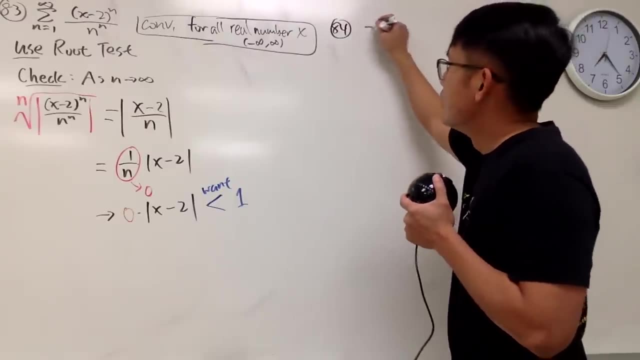 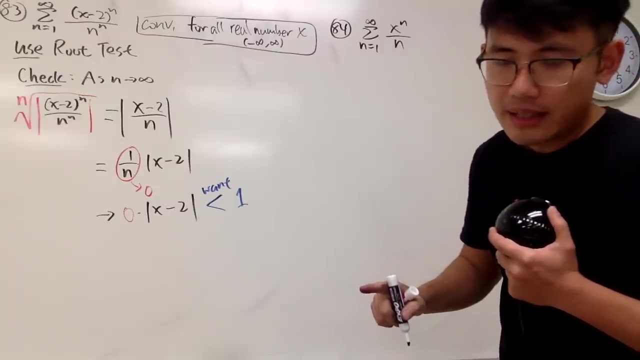 You'll see. All right now number 84.. We are going to do the same thing. Sum as n goes from 1 to infinity, x to the n over, just an n. all right, And then, yeah, I want to see: when does this converge? 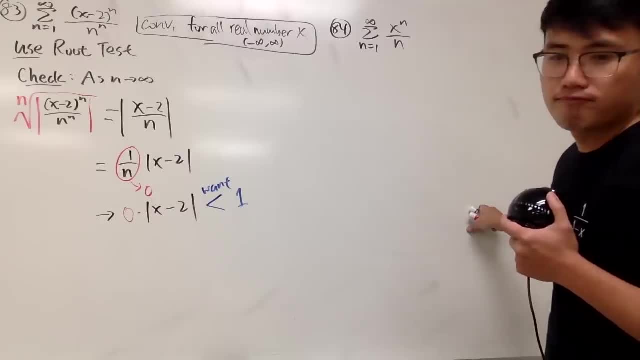 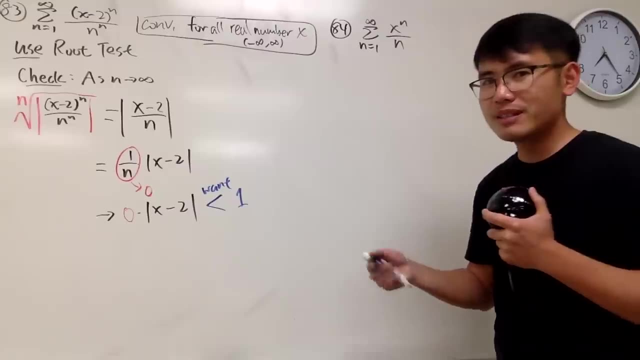 Huh, Well, if you do the root test, I think it's still OK, because we know how to handle that. But now let me show you guys how you use the ratio test, And earlier you could have used the ratio test as well, right? 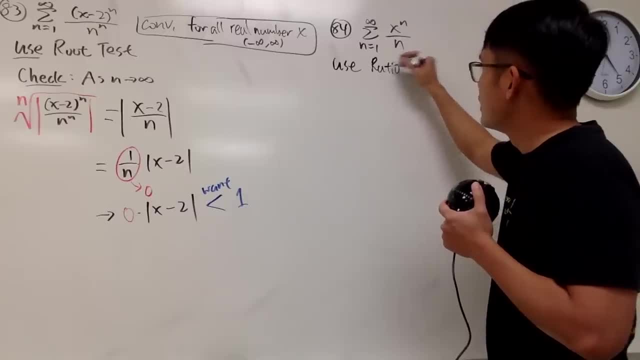 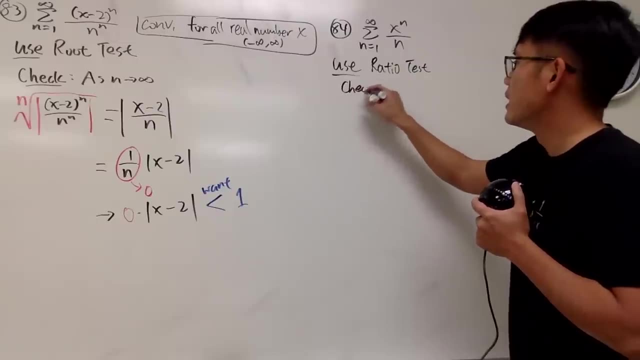 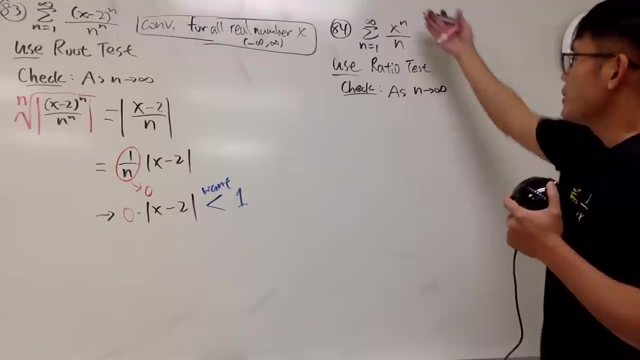 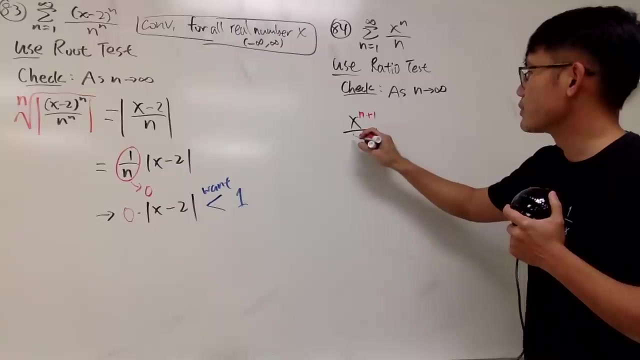 So let me just say: use the ratio test. Now, here is the deal: Check the limit as x, so as n goes to infinity, Ratio test in action. here we have x- I don't know what it is yet- and then you raise that to the n plus 1 power, and then you divide it by n plus 1, right here, right. 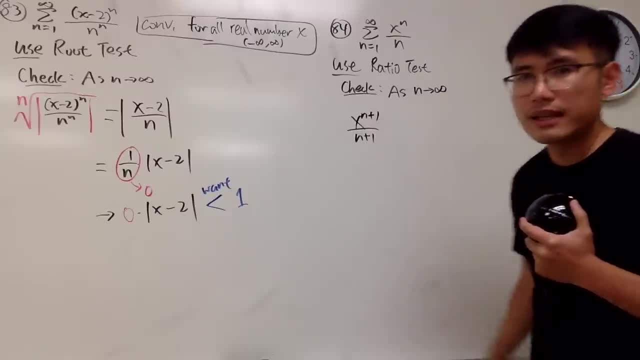 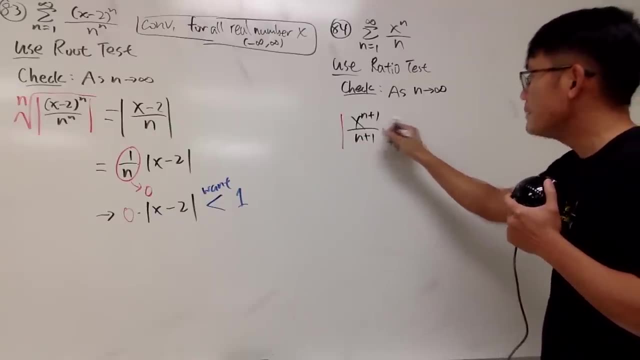 x, n plus 1 over n plus 1, like this and like that. OK, don't forget the absolute value. It's needed, especially if you don't want x's Times n over x to the n, like that. 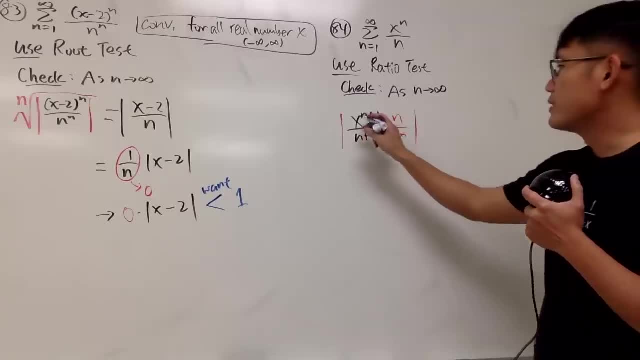 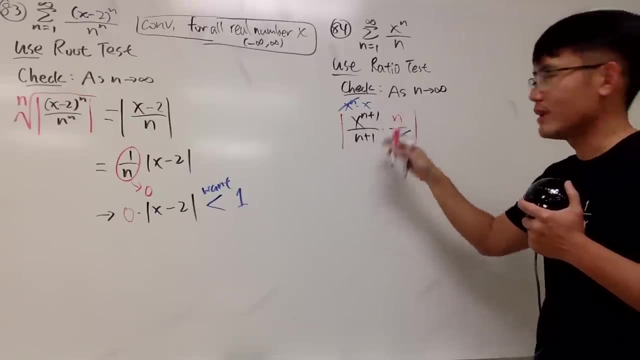 OK, OK, OK, OK, OK, OK, OK. Do the usual thing. This right here is x to the n times x. Cancel this guy out, so we have the x by itself right here. So here's the deal. 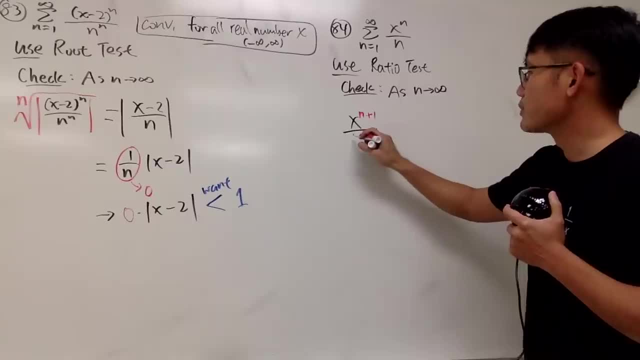 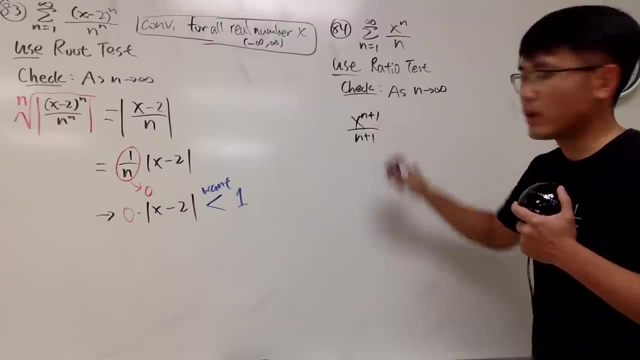 to the m plus one power and then you divide it by m plus one right here, right x m plus one over m plus one, like this and like that. Okay, don't forget the absolute value It's needed, especially if you don't want x's. 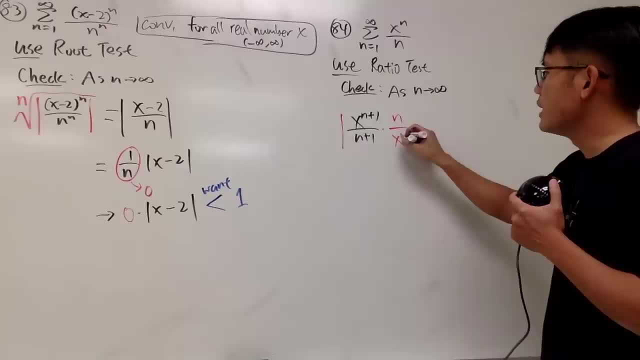 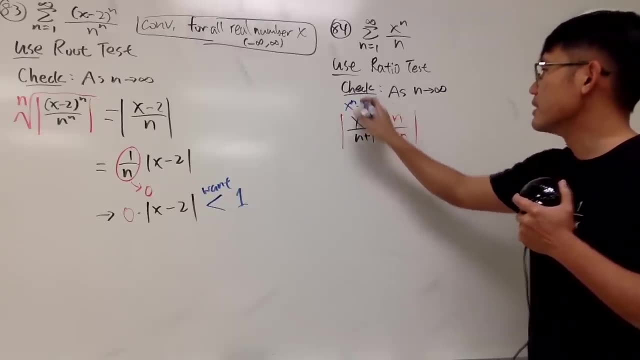 Times n over x to the n, like that. Now do the usual thing. This right here is: x to the n times x. Cancel this guy out, so we have the x by itself right here. Then we'll have the n's. 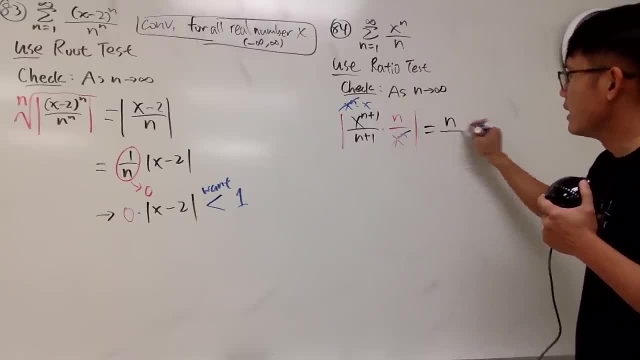 So here's the deal: n and n plus 1, they are good to go on the outside, But the absolute value of x has to be inside here And you want this to be less than 1 after you take the limit. 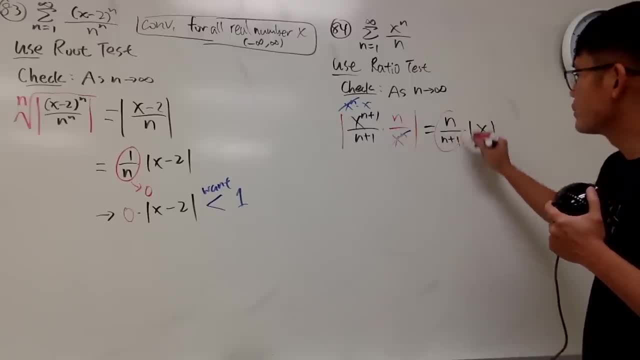 So let's do that right here. And when you take the limit, this right here- n over n plus 1, will give you the limit equal to 1.. So this right here is 1 times the absolute value of x, like this: 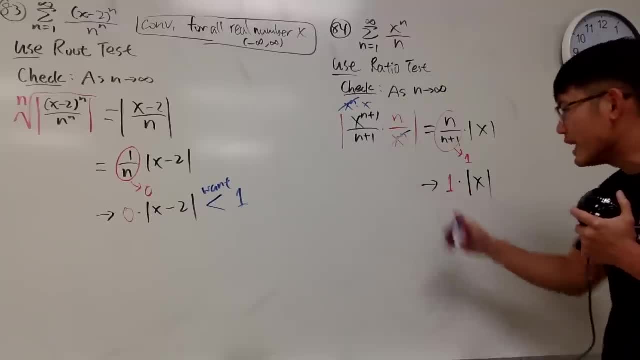 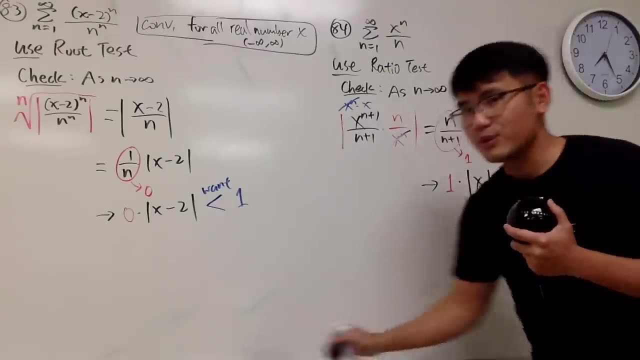 So this is the result after the ratio test. all that, But again, just like this, we want to set- or I'll just say we want or set, doesn't really matter same thing- We want to set this to be less than 1.. 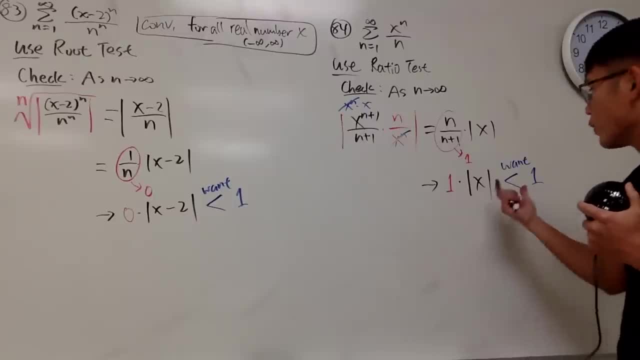 So now we have an inequality. This sets a condition of like. when does this have to be true, right? So this, right here, of course, 1 is just that. so it's just: absolute value of x is less than 1.. 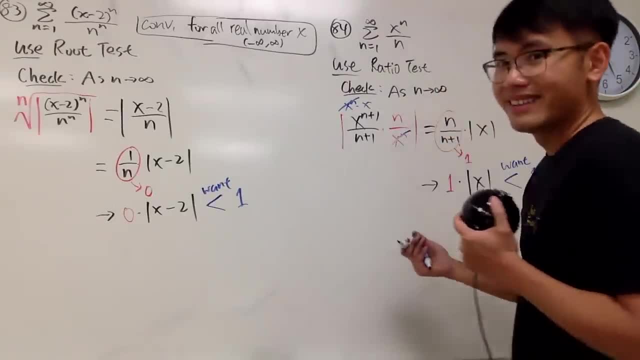 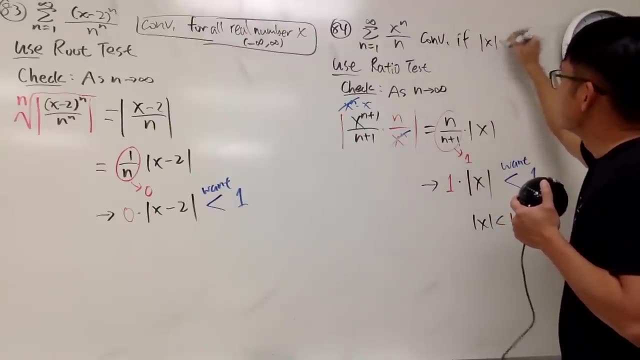 So this is kind of like saying: to find the condition for the best friend, To find the condition for the best friend. This right here converges if the value of x is less than 1.. In another word, x has to be less than. 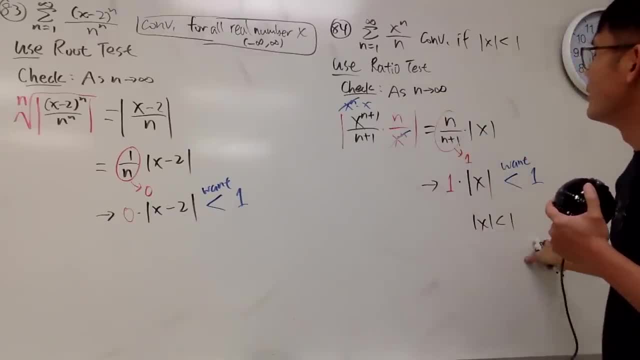 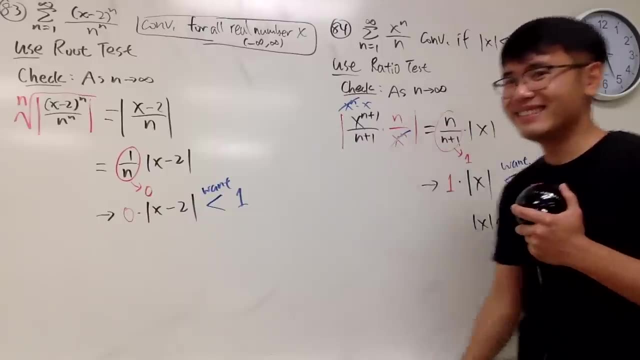 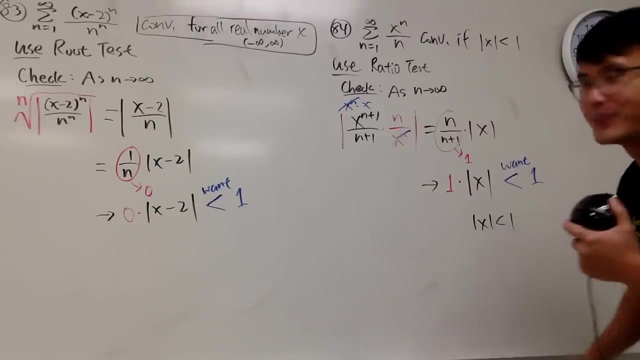 x has to be in between of negative 1 and 1.. Oh, I see, Okay, Okay, Okay, Huh, Okay, okay, okay. I forgot to do this, but thank God this right here. the radius of convergence is just infinity, so it doesn't really matter. 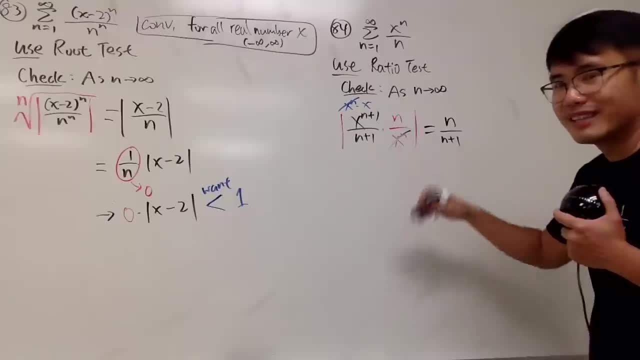 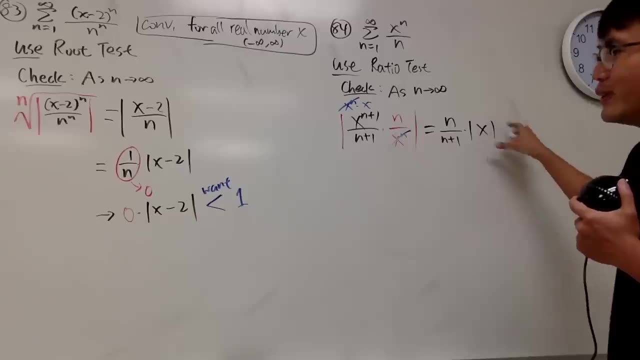 n and n plus 1, they are good to go on the outside, But the absolute value of x has to be inside here, And you want this to be less than 1 after you take the limit. So let's do that right here. 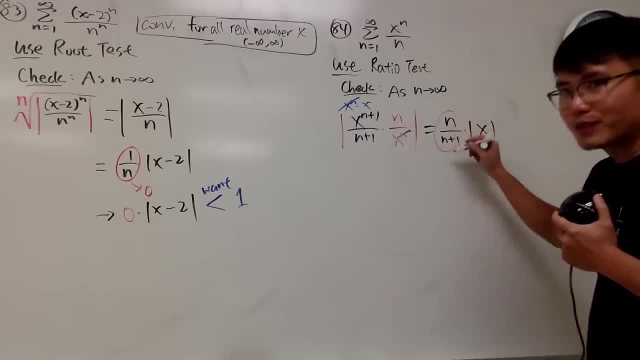 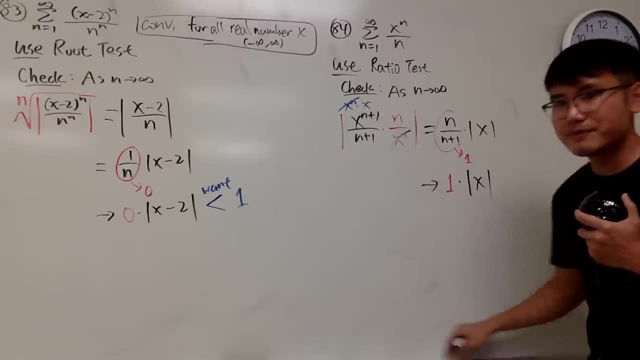 And when you take the limit, this right here, n over n plus 1 will give you the limit equal to 1.. So this right here is 1 times the absolute value of x, like this. So this is the result after the ratio test. all that: 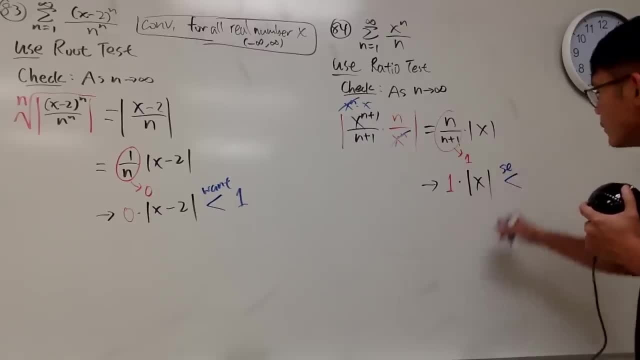 But again, just like this, we want to set- or I'll just say we want to set, doesn't really matter same thing. We want to set this to be less than 1.. So now we have an inequality. This sets a condition of like. when does this have to be true, right? 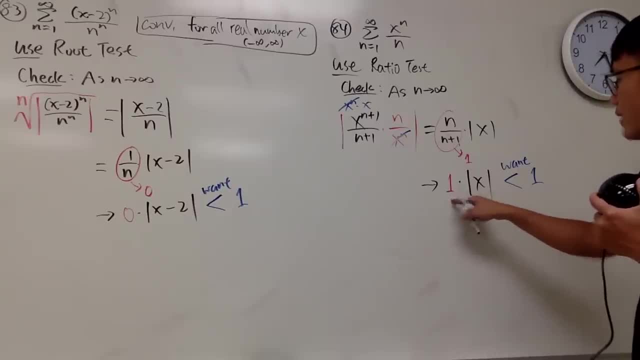 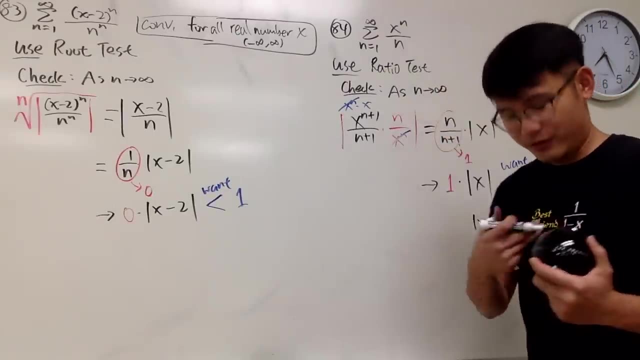 So this right here, of course, 1 is just that. so it's just absolute value of x is less than 1.. So this is kind of like saying: to find the condition for the best friend, Find the condition for the best friend. 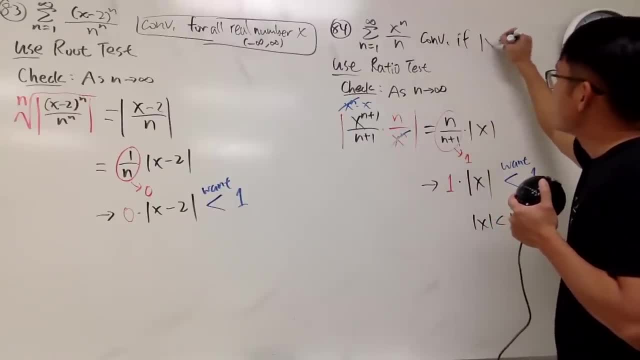 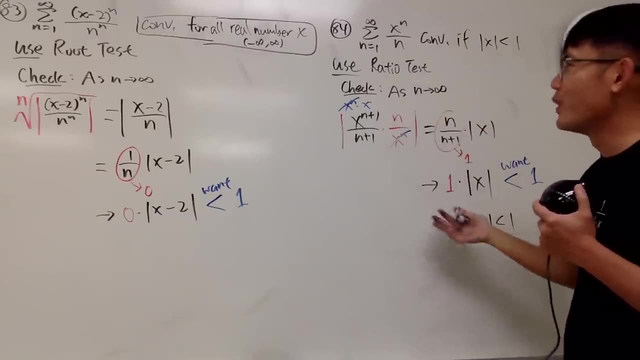 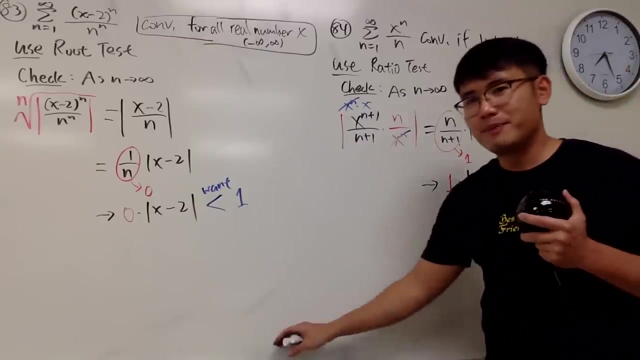 This, right here, converges if absolute value of x is less than 1.. In other words, x has to be less than x has to be in between of negative 1 and 1.. Oh, I see, Okay, Okay, Okay. 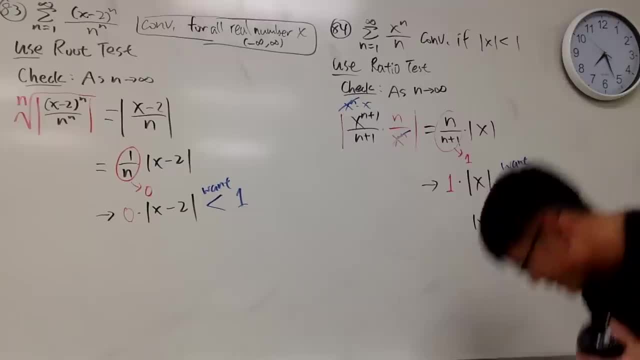 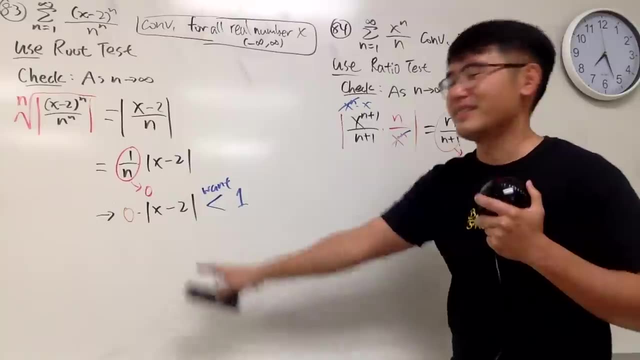 Huh, Okay, okay, okay, I forgot to do this, but thank god, this right here. the radius of convergence is just infinity, so it doesn't really matter, right, But you have this right here. so we have to do the following. 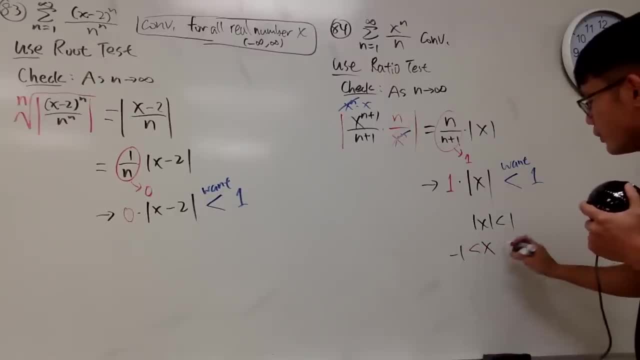 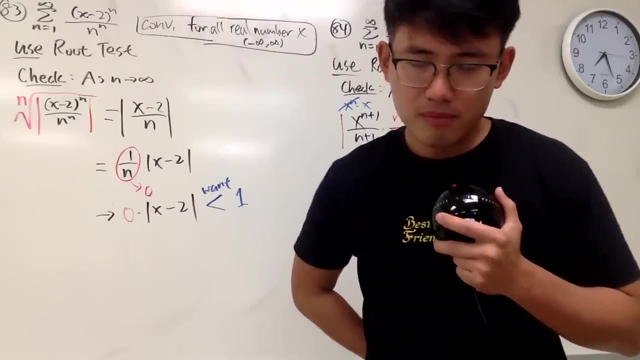 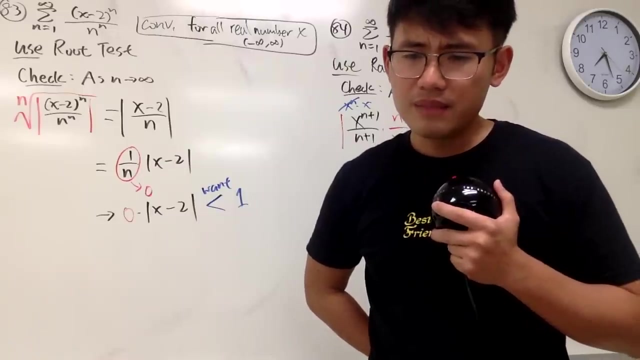 It seems like I could have done. x is in between of negative 1 and 1, like that. It seems like I could have done. x is in between of negative 1 and 1, like that, Earlier. yeah, well, number 82 was the best friend, so that you don't include the endpoints. 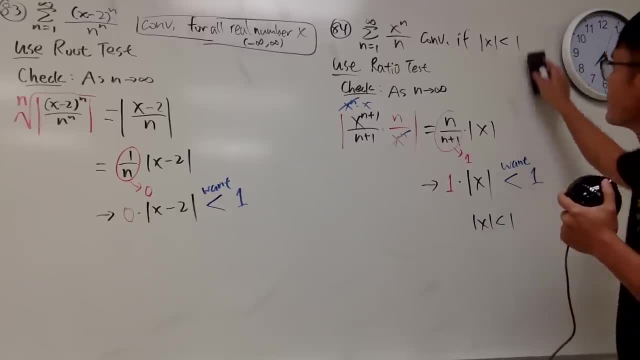 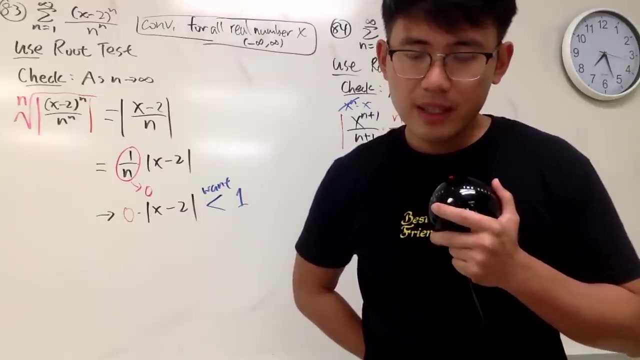 But you have this right here. So we have to do the following. It seems like I could have done x's in between of negative 1 and 1, like that, Earlier. yeah well, number 82 was the best friend. 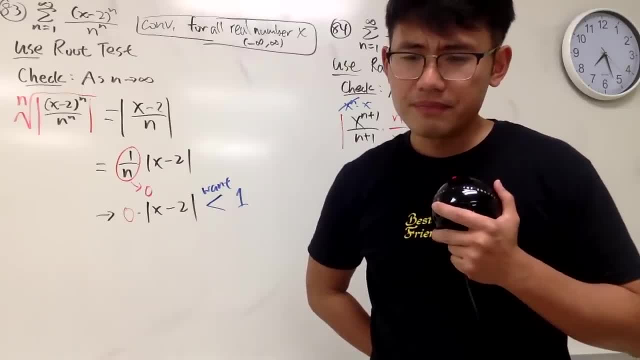 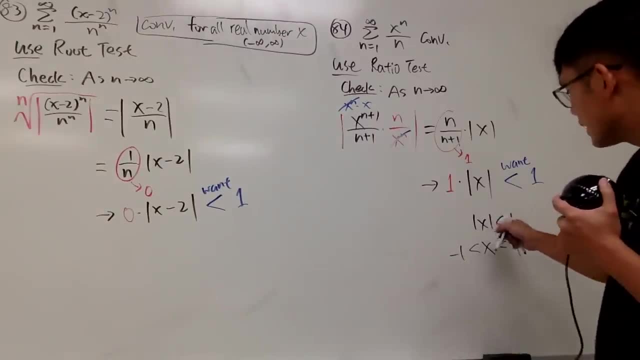 So that you don't include, you don't include that, you don't include the endpoints, But it seems like, It seems like, once I get to this, what happens to this right? So it seems like I can just go from here to here. 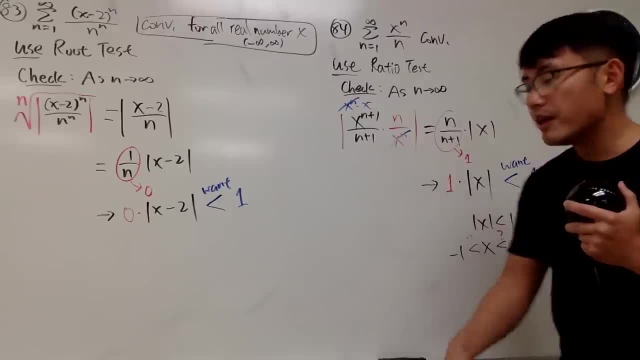 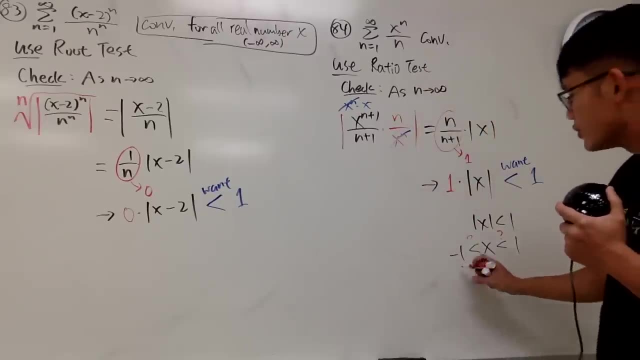 But now here is the deal You have to remember if you are doing this kind of things: to find the radius of convergence for the power series, you will have to check what if x is exactly negative 1 and also what if x is exactly 1.. 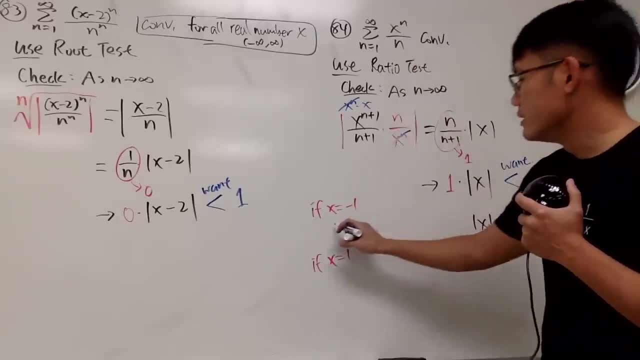 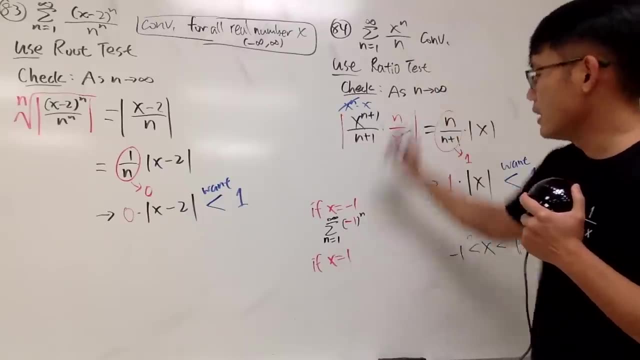 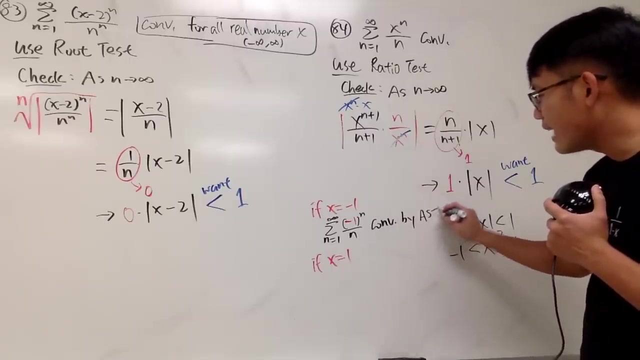 So let's do that real quick. If x is exactly negative 1, this is the sum as n goes from 1 to infinity negative 1 to the nth power over n. This right here actually converges by AST. So at the endpoint sometimes we have a chance. 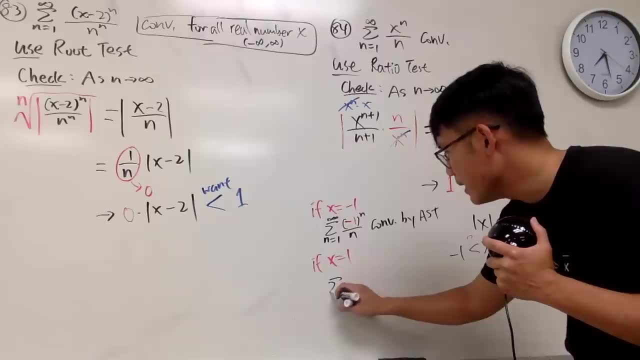 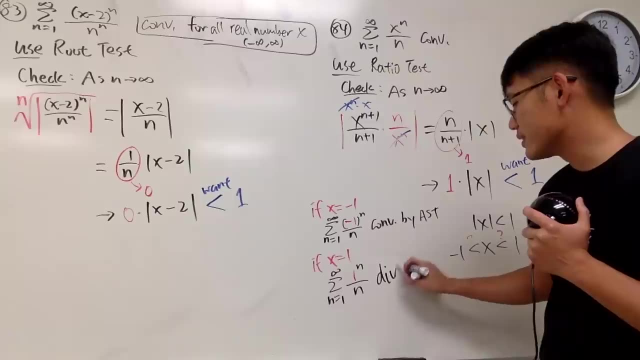 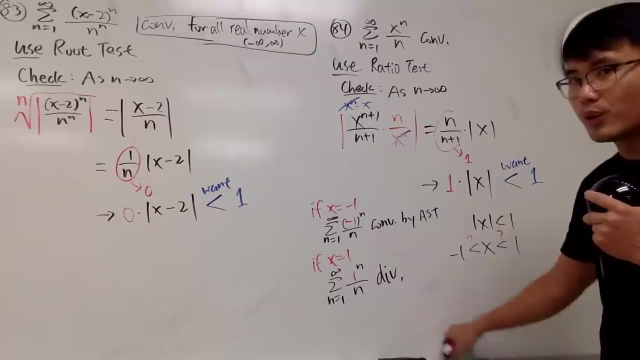 Right here, when we put in 1, we get the sum as n goes from 1 to infinity, We have 1 to the nth power over n. This right here is divergent because we have done it so many times. So the truth is you don't know this yet unless you do the work to check. 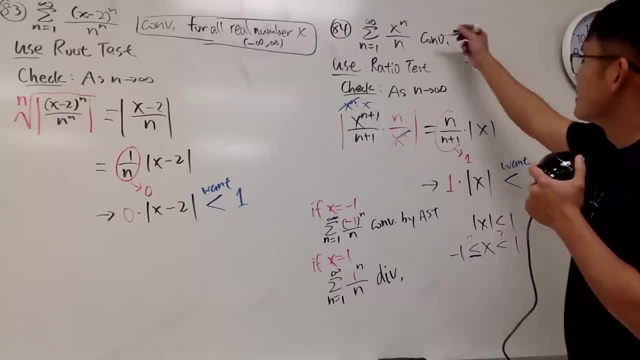 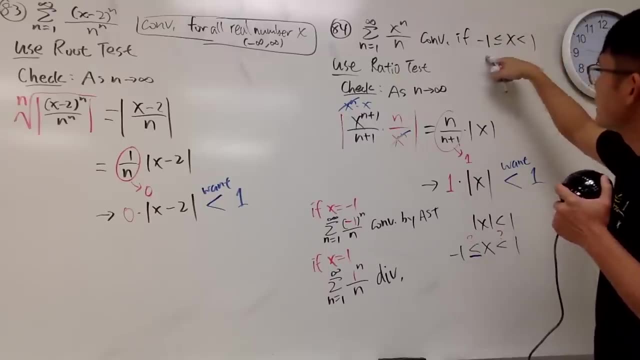 So you have to include that. So converges, if I will just put on the inequality there, Negative 1, less than or equal to x and then less than 1.. x is in between negative 1 and 1.. But including negative 1, not positive 1.. 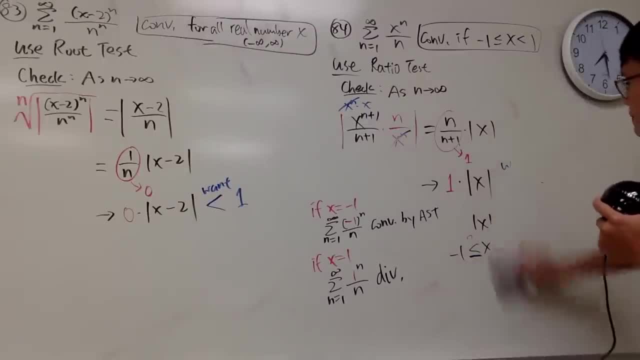 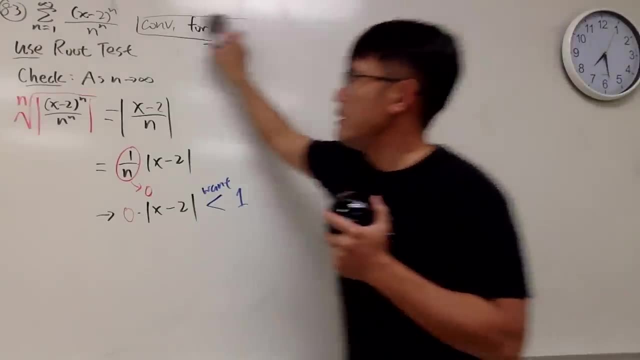 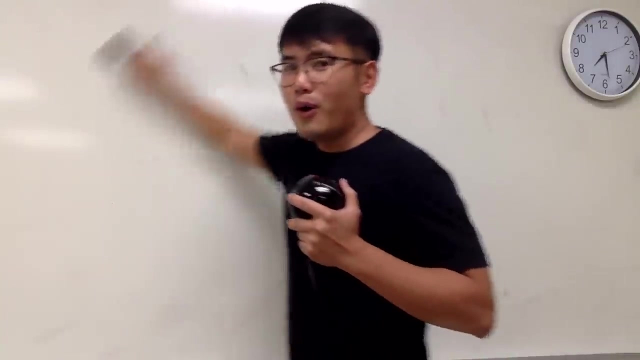 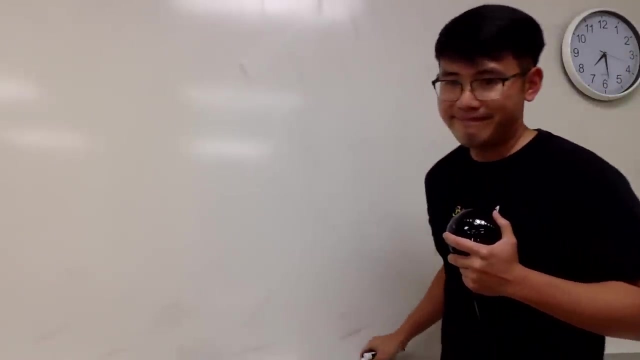 So it's just like this: I feel like going on a strike already. It's like, okay, you guys are on your own. Bye everybody, Happy Sunday. It's okay, though I will not leave you guys behind. Let's see what's next. 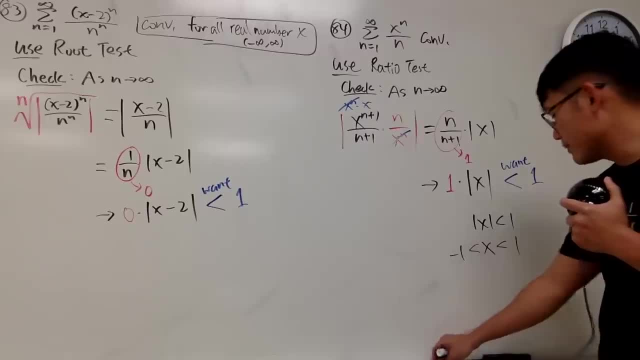 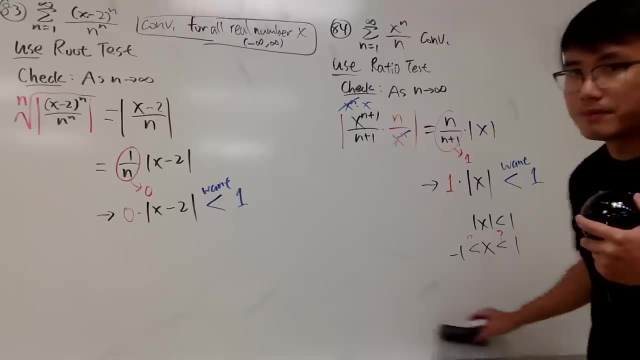 But it seems like once I get to this, what happened to this right? So it seems like I can just go from here to here. but now here is the deal You have to remember if you are doing this kind of things. 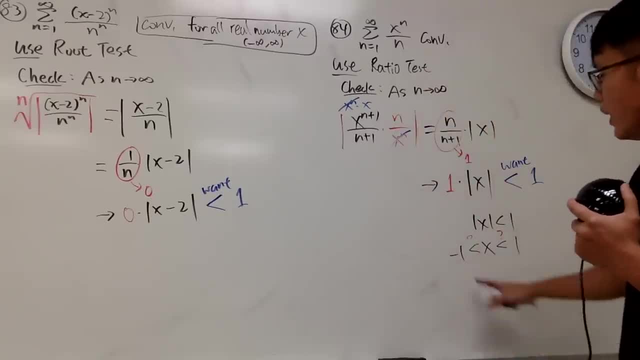 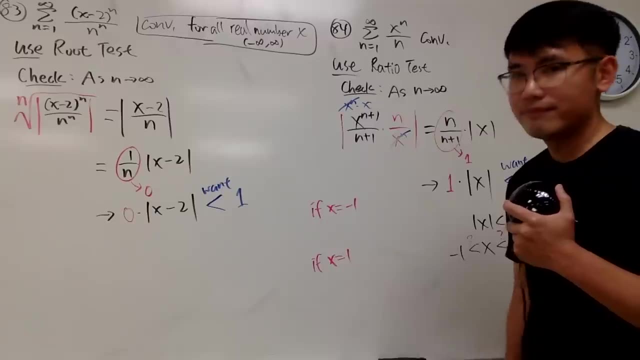 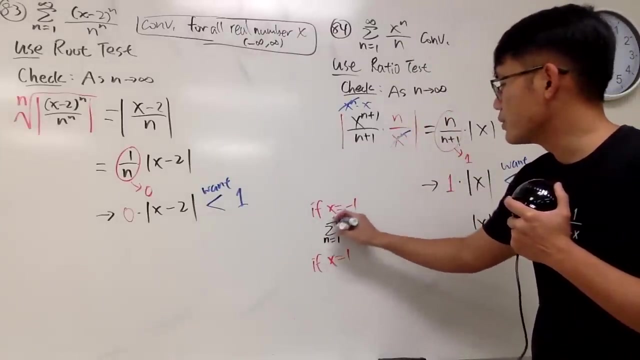 to find the radius of convergence for the power series, you will have to check what if x is exactly negative, 1, and also what if x is exactly 1.. So let's do that real quick. If x is exactly negative, 1,. this is the sum as n goes from 1 to infinity. 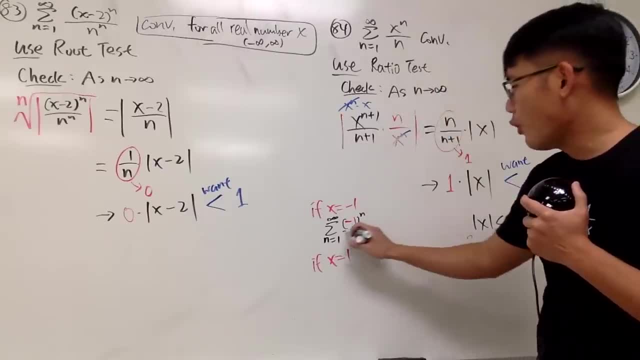 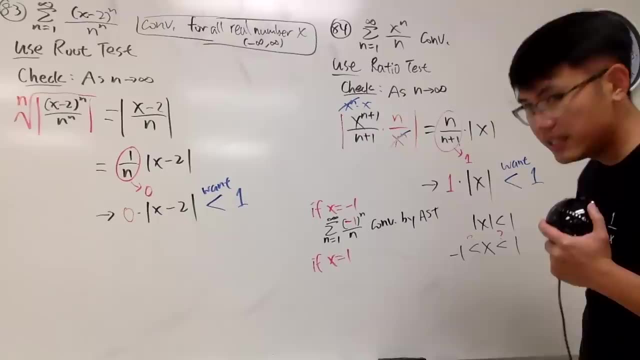 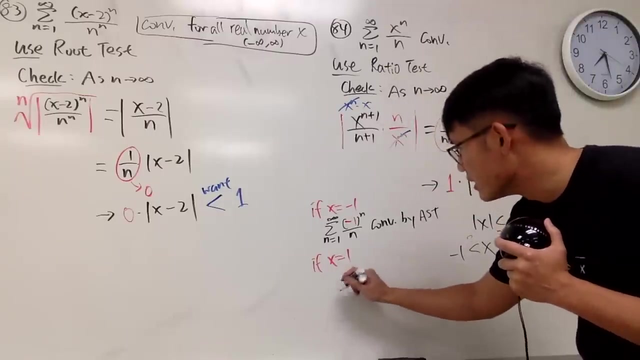 negative. 1 to the x, to the nth power. sorry over n. This right here actually converges by a s, t. Okay, So at the endpoint sometimes we have a chance Right here, when we put in 1, we get the sum as n goes from 1 to infinity. 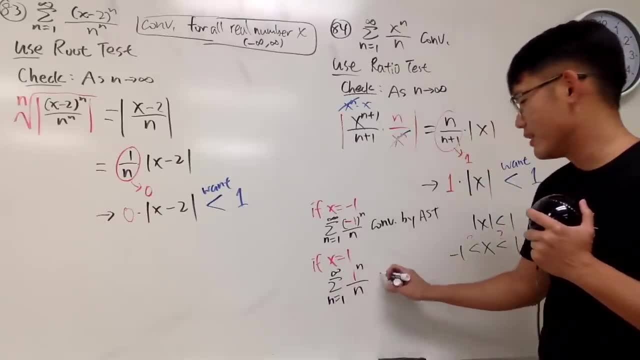 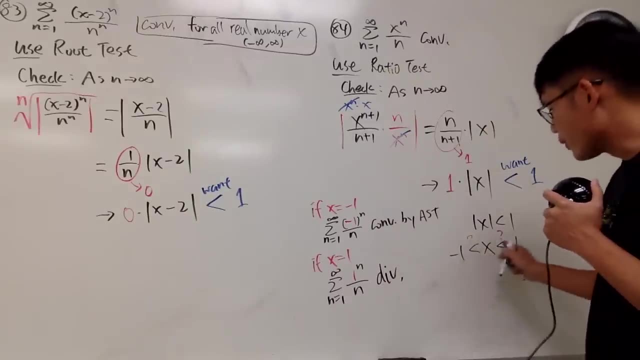 We have 1 to the nth power over n. This right here is divergent because we've done it so many times. So the truth is you don't know this yet unless you do the work to check. so you have to include that. 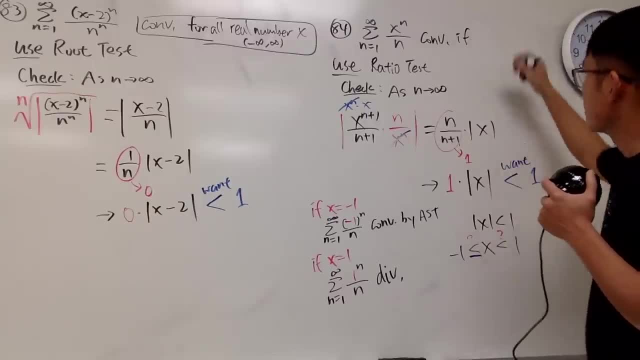 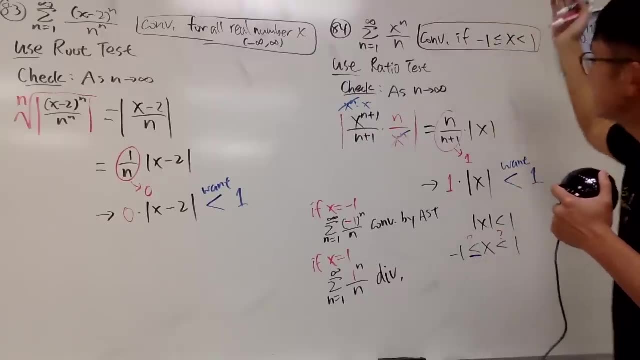 So converges. if I will just put on the inequality there: negative 1 less than 1.. We go to x and then less than 1.. x is in between negative 1 and 1, but including negative 1, not positive 1.. 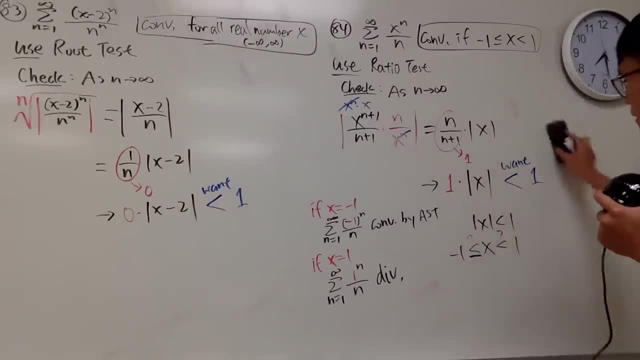 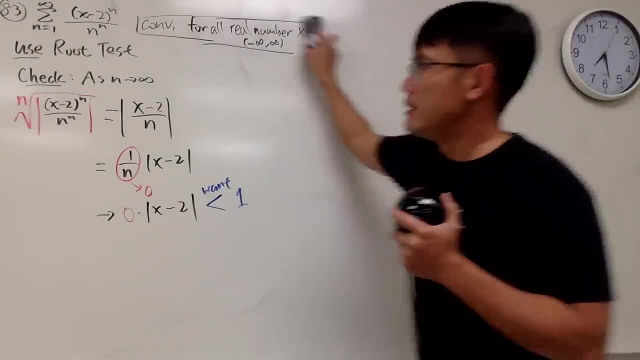 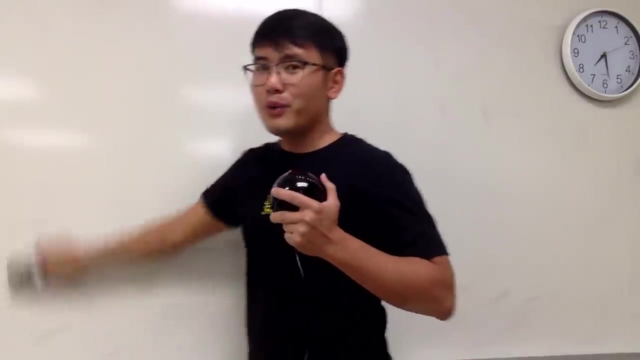 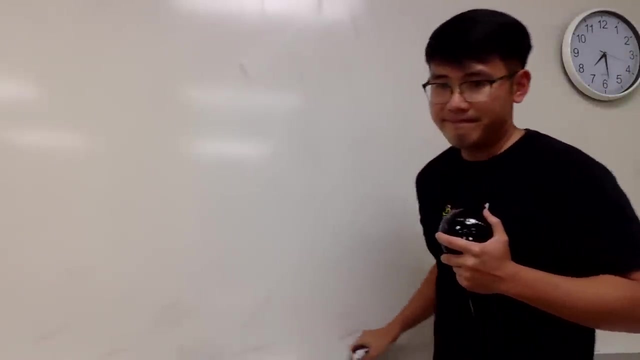 So it's just like this: All right, I feel like going on a strike already. It's like, okay, you guys are on your own. Bye everybody, Peace Sunday. It's okay, though I will not leave you guys behind. 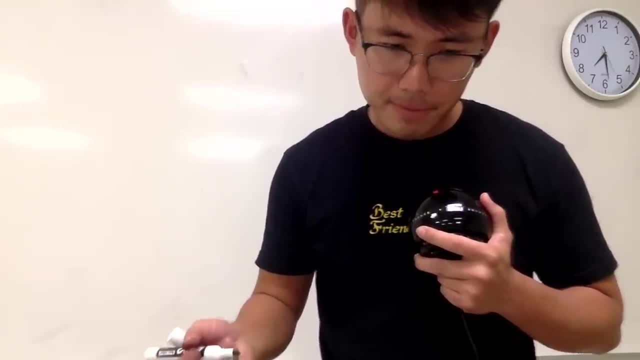 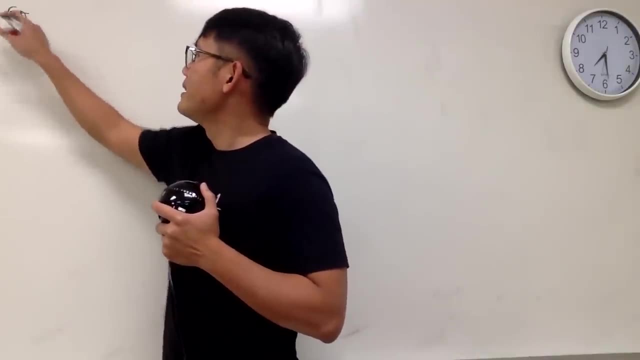 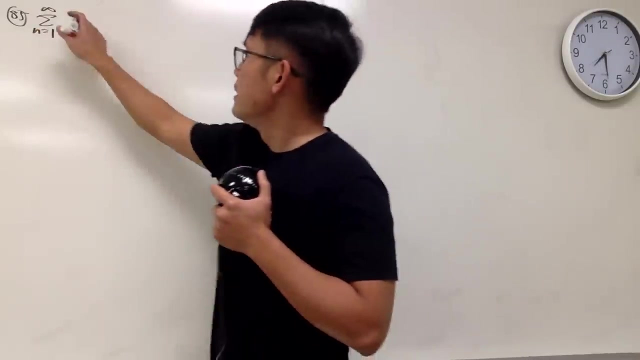 Let's see what's next. Okay, Number 85.. Right here, This question takes some time, man. The sum as n goes from 1 to infinity, And we have x minus 1 to the nth power over, And we have n times 3 to the nth power. 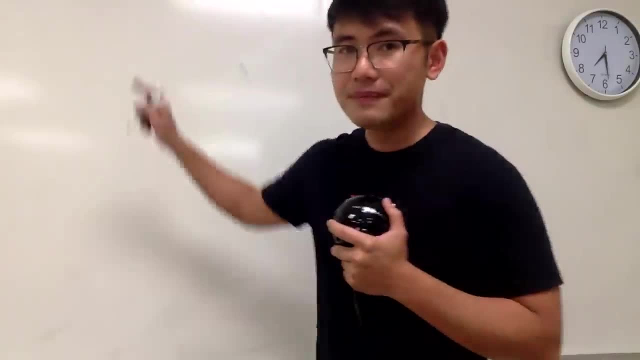 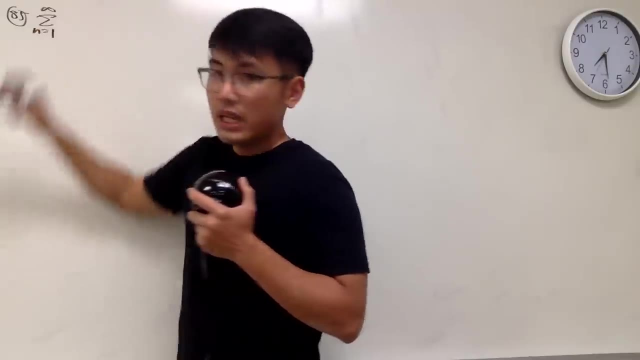 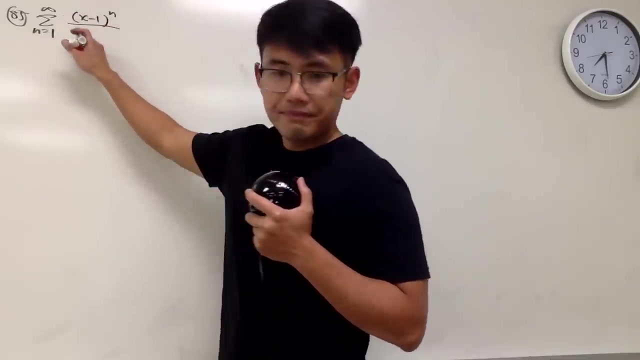 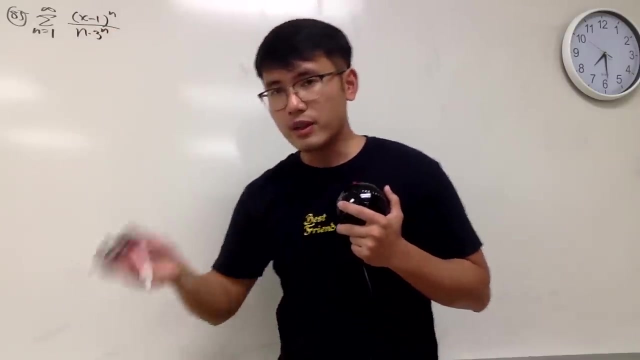 Okay, number 85.. Right here, This question takes some time, man. The sum as n goes from 1 to infinity And we have x minus 1 to the nth power, over n times 3 to the nth power. So here's the deal. 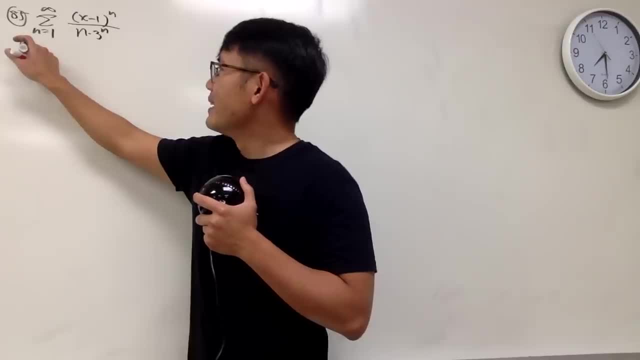 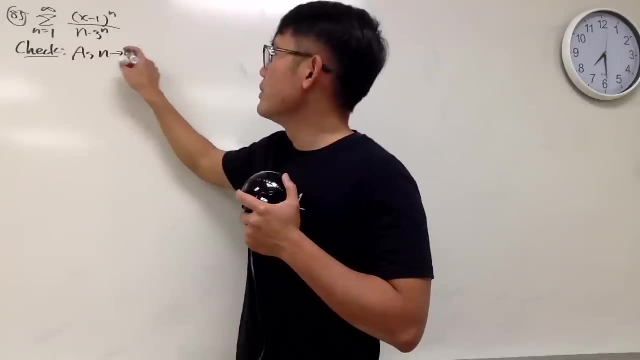 Just use the Rieser test, Much better, So yeah. So I will just say: use the Rieser test. Okay, So we'll check. As n goes to infinity ratio test in action. x is just x, You don't touch it. 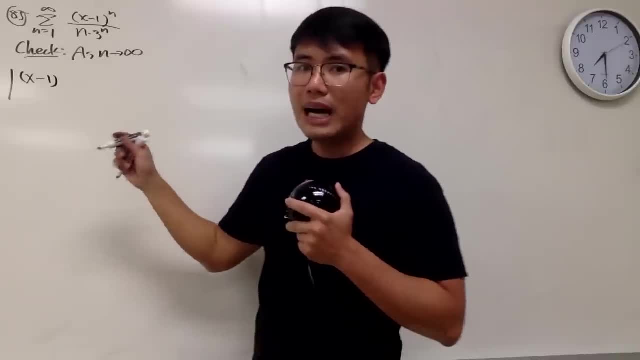 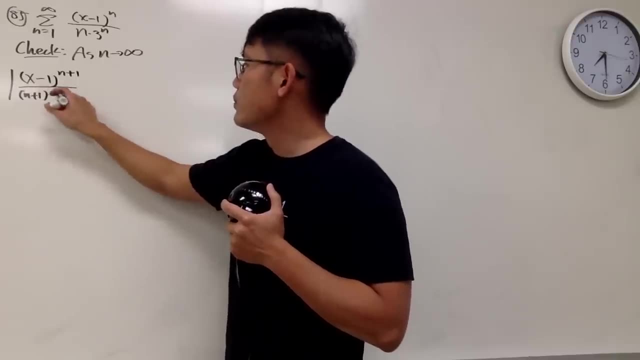 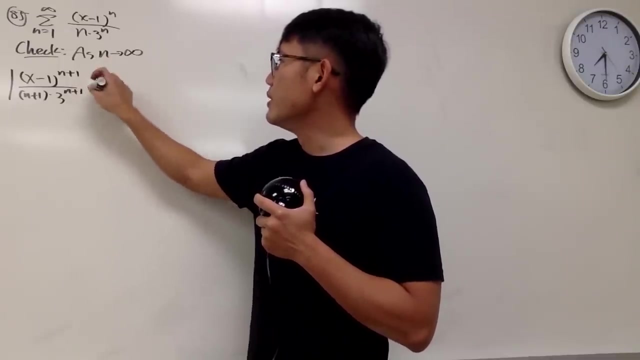 So you have x minus 1.. And there you have n plus 1, power now over n plus 1 times 3 to the n plus 1.. Like this. And then you are going to multiply by the reciprocal, which is n times 3 to the nth. 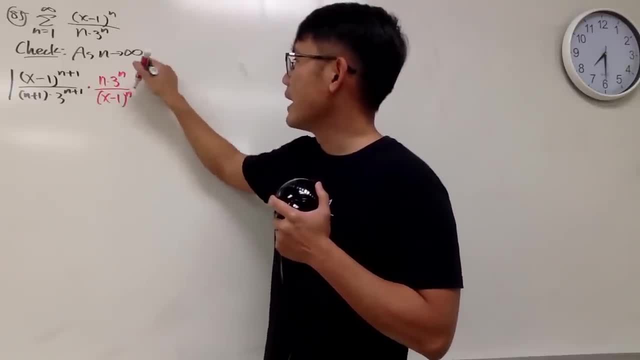 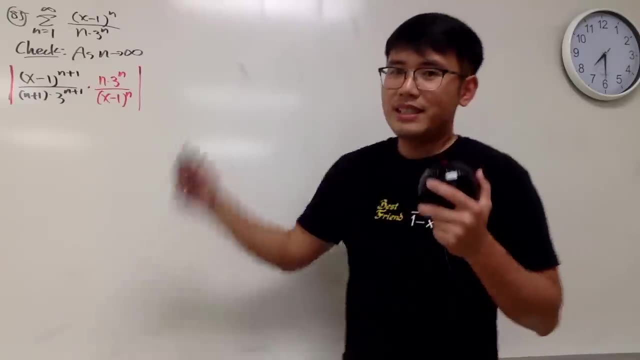 And then over x minus 1 to the nth power, like that, Of course, absolute value for the Rieser test. Now just let's see what we can cancel out right Here. this is 3 to the n times 3 to the first. 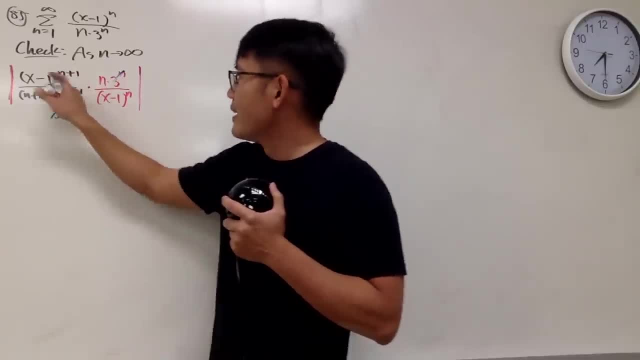 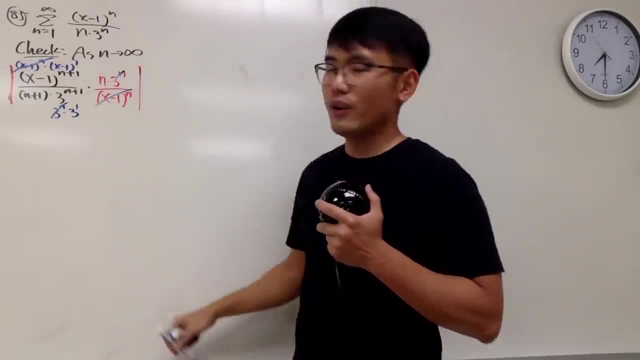 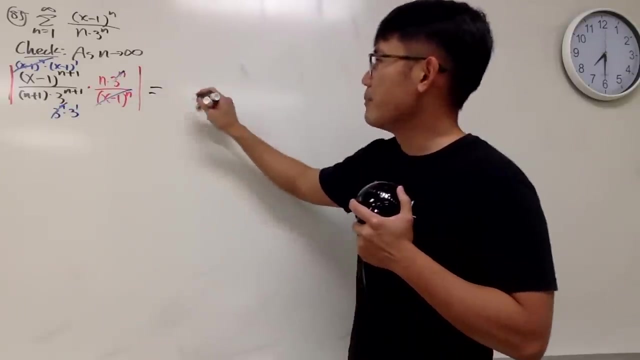 This that cancel, That's good. Here, you know, this is x minus 1 to the n, times x minus 1 to the 1.. This that cancel, That's nice Good. Okay, n over n plus 1 can be come out, because they are all positive. 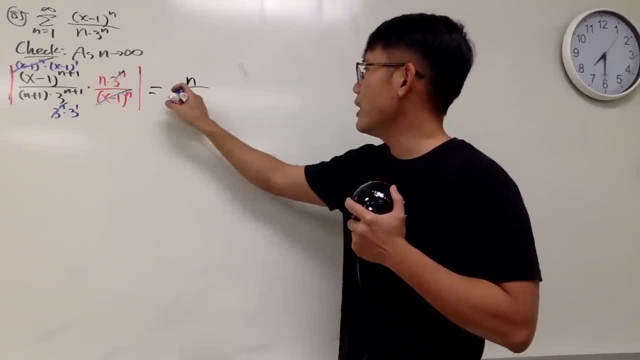 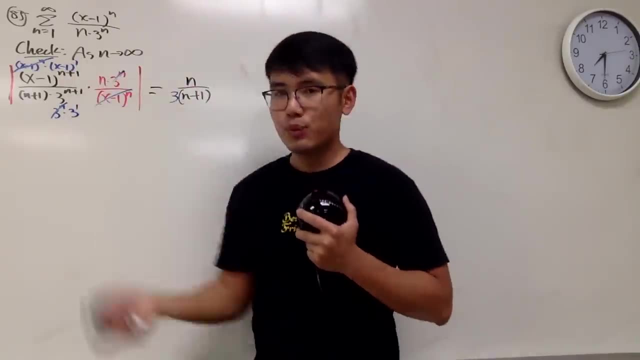 And don't forget, we still have the 3 as well. So perhaps I'll put that down a little bit in red and in blue. And then we have the n plus 1, like that x minus 1 to the first power. 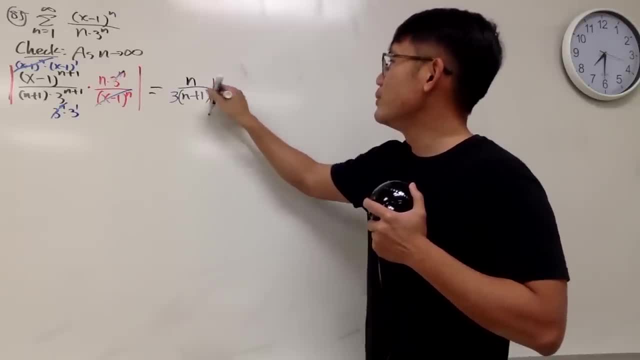 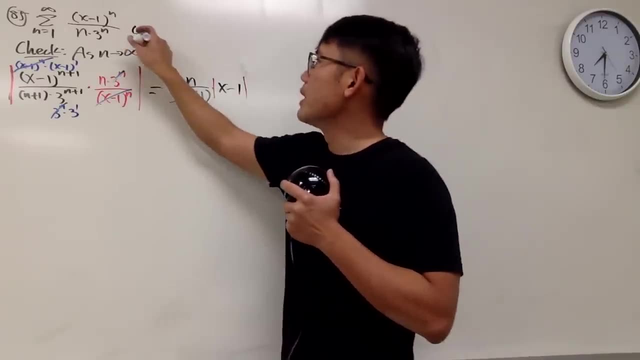 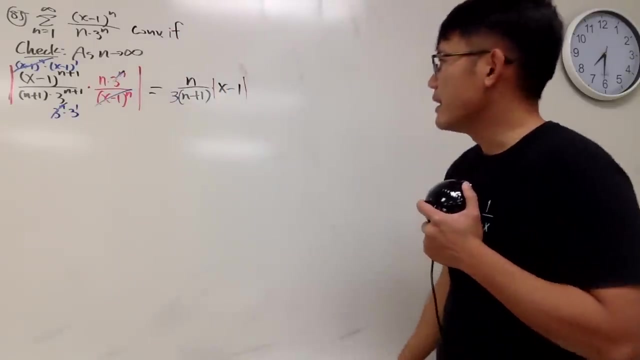 that's what we have to maintain in the absolute value x minus 1, because we don't know what x is yet We have to find it. So let me, let me just put down: converge if and converge if. Okay, Now let's take the limit, as n goes to infinity. 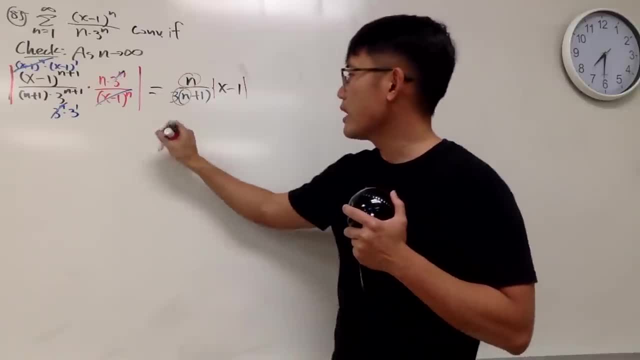 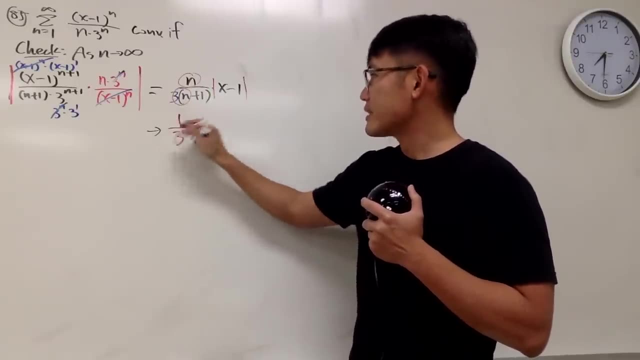 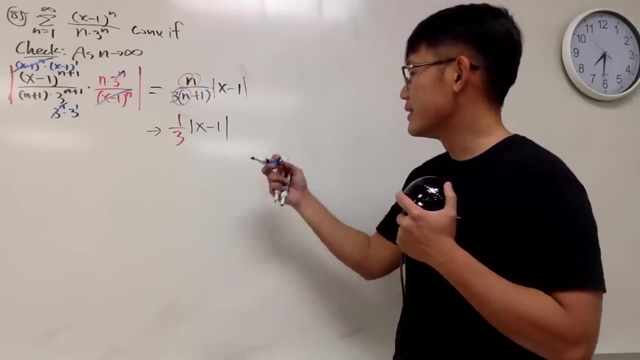 We know, care about this, care about that. So all in all we end up with 1 third for the limit right here times the absolute value of x minus 1.. And then you know the deal We are going to set this right. 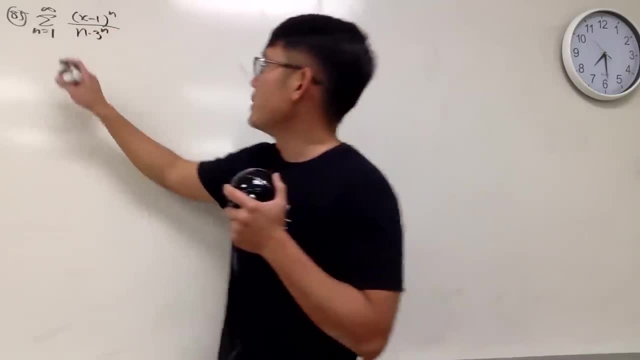 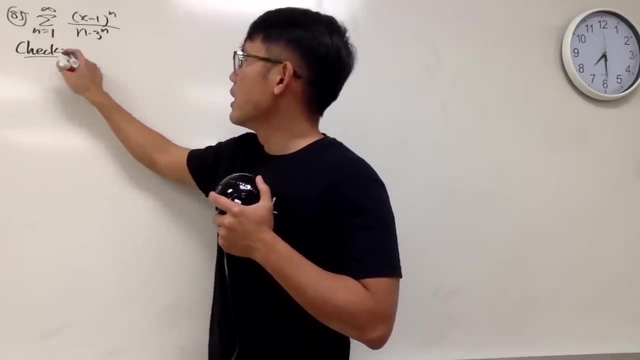 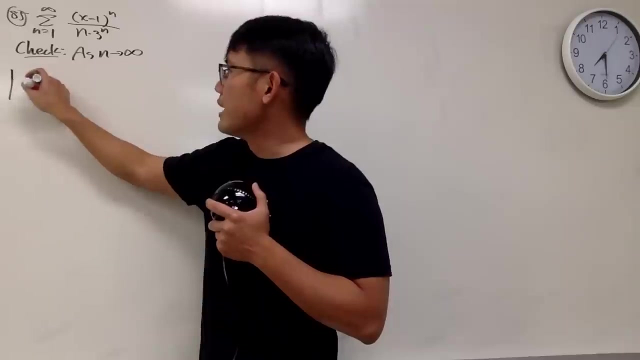 So here's the deal: Just use the ratio test, Much better. So I will just say: use the ratio test, okay, So we'll check. S? n goes to infinity Ratio test in action. x is just x, You don't touch it. 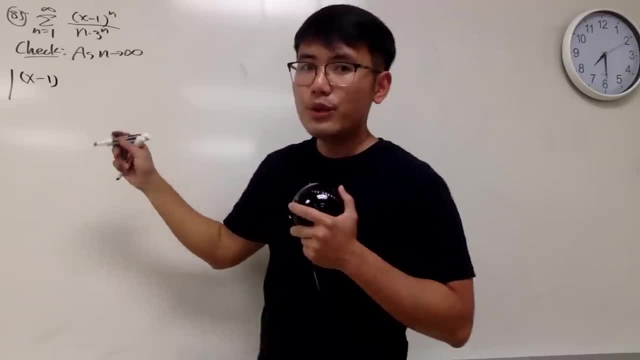 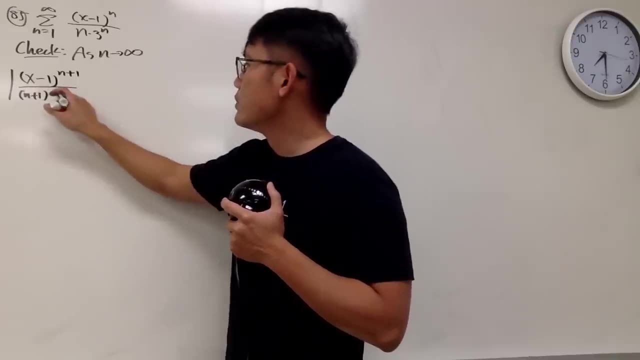 So you have x minus 1.. And there you have n plus 1 power. now All for infinity, All for infinity, All for infinity, Over n plus 1 times 3 to the n plus 1.. Like this, And then you are going to multiply by the reciprocal. 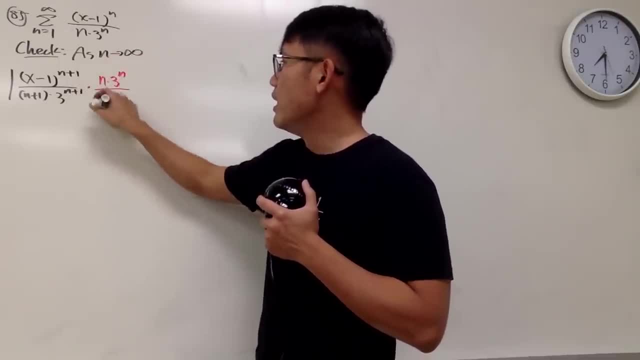 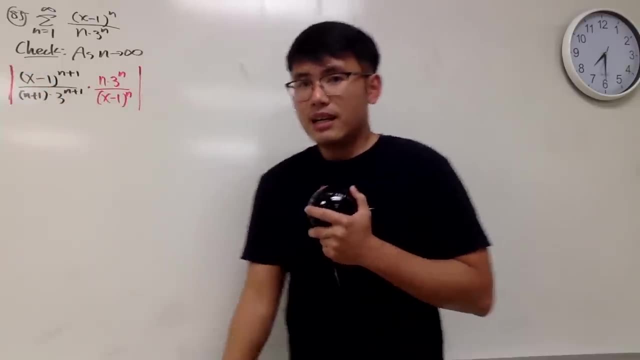 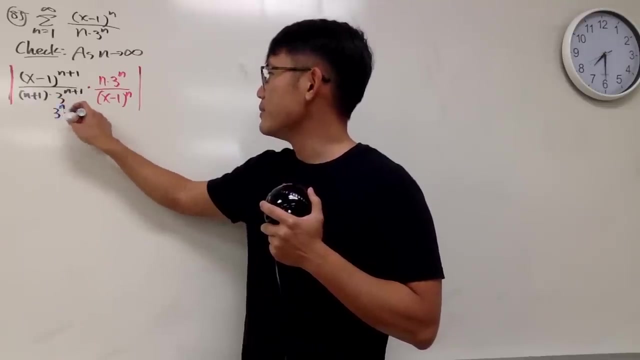 which is n times 3 to the n over x, minus 1 to the nth power. Like that, Of course, absolute value for the ratio test. Now just let's see what we can cancel out right Here. This is 3 to the n times 3 to the first. 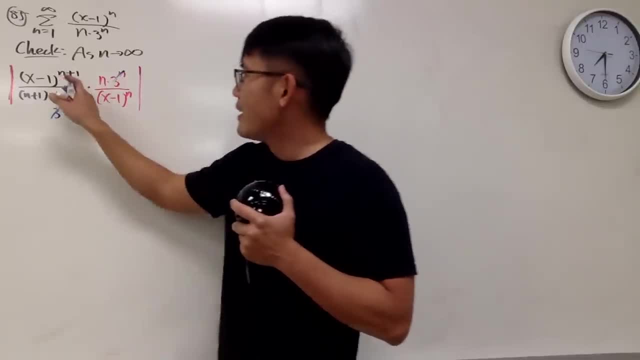 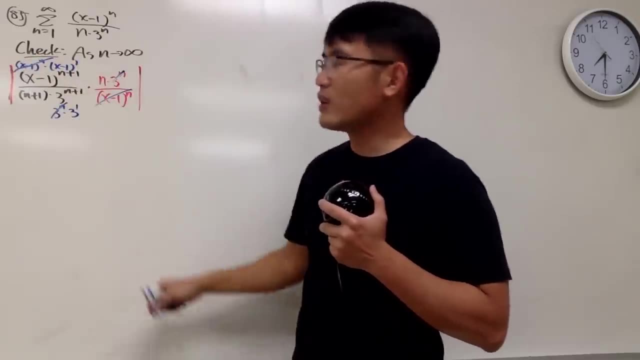 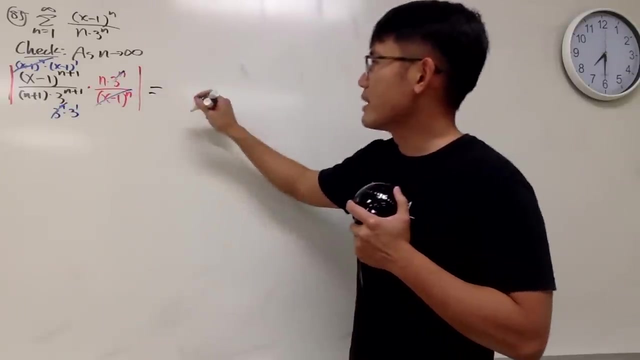 This That Cancel, That's good. Here, You know, this is x minus 1 to the n, times x minus 1 to the 1. This That Cancel, That's nice Good. Okay, n over n plus 1 can be come out, because they are all positive. 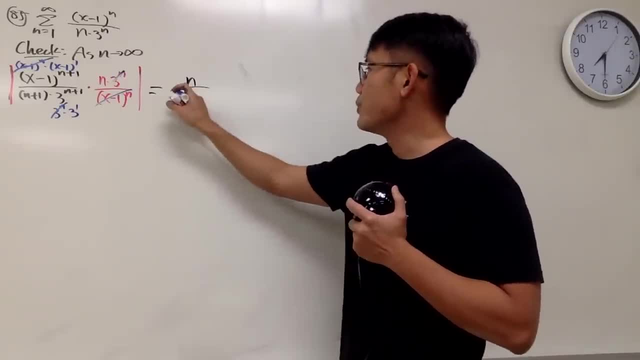 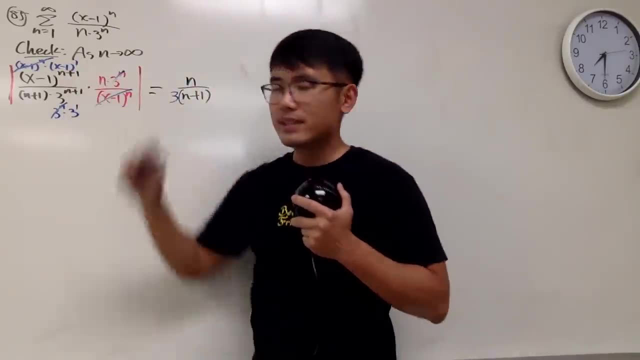 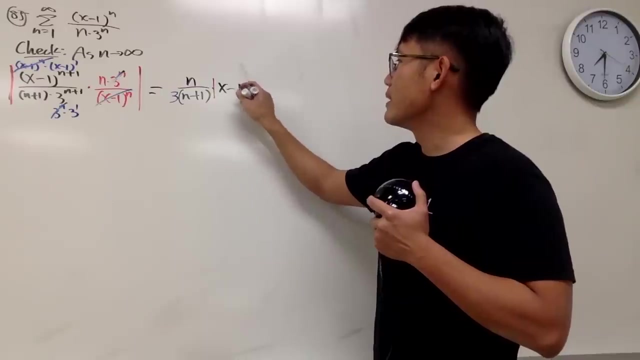 And don't forget, we still have the 3 as well. So perhaps I'll put that down a little bit in red and in blue. And then we have the n plus 1, like that, But x minus 1 to the first power. that's what we have to maintain in the absolute value x minus 1.. 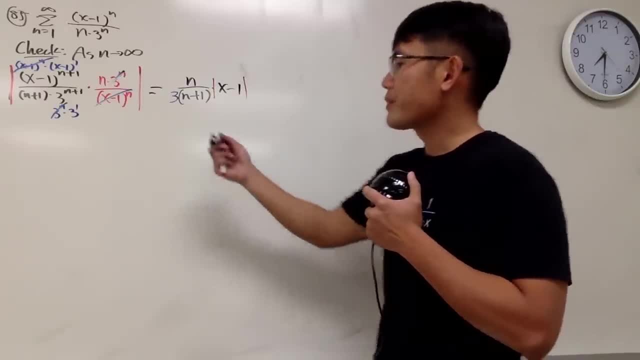 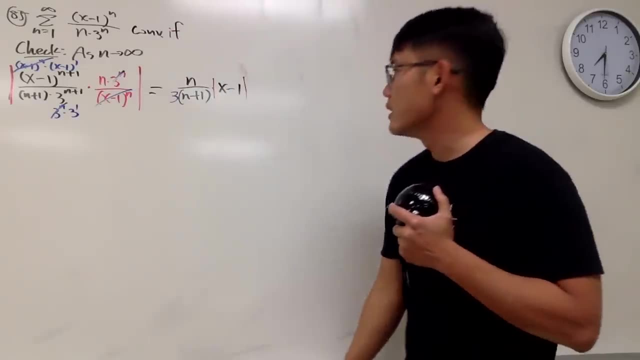 Because we don't know what x is yet We have to find it. So let me just put down: converge if, Converge if. Okay, Now let's take a limit, as n goes to infinity. We know, care about this, care about that. 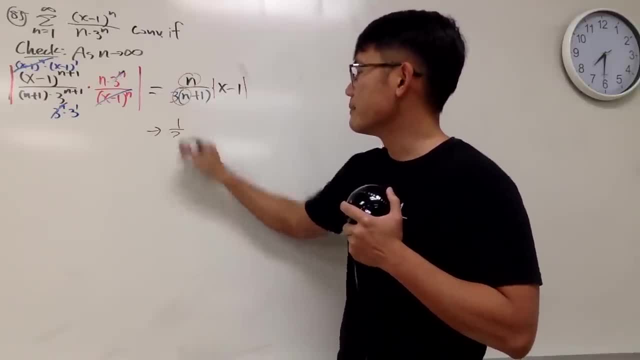 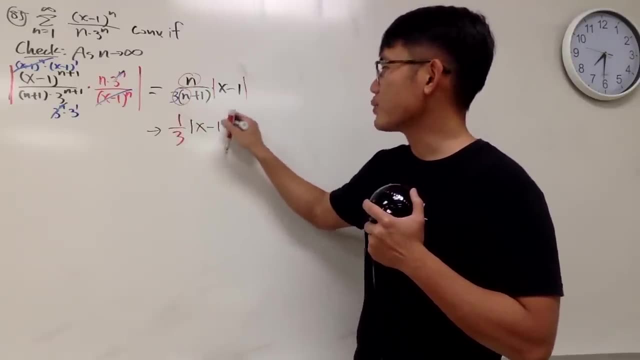 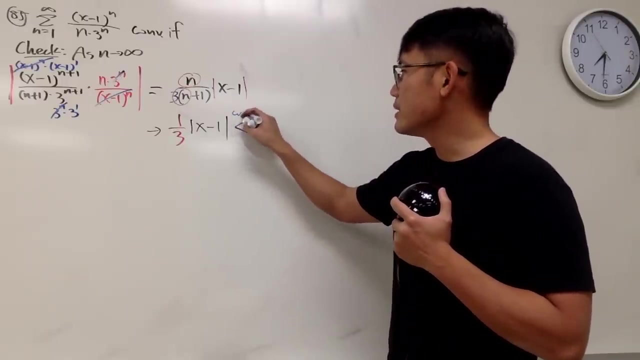 So all in all, we end up with 1 third for the limit. Right here Times the absolute value of x minus 1.. And then you know the deal We are going to set this right: We want this to be less than 1.. 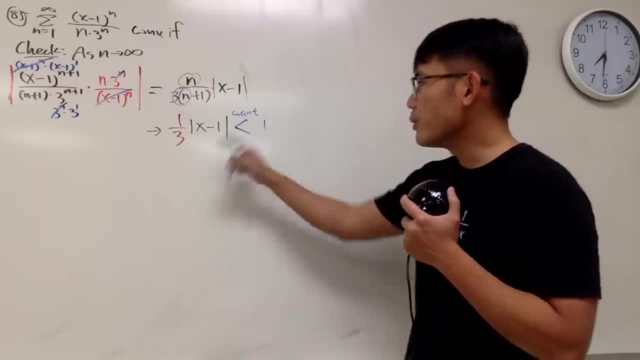 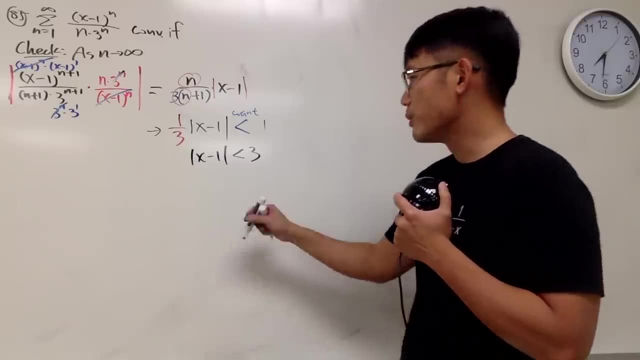 And now let's just play around with this inequality. Multiply by 3 on both sides, So we get the absolute value of x minus 1 is less than 3.. And of course you can do a little bit. This is just x minus 1.. 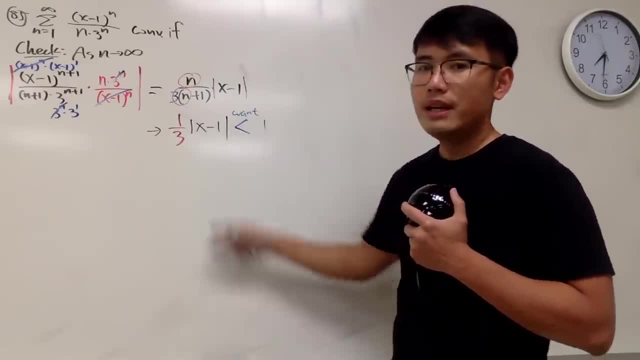 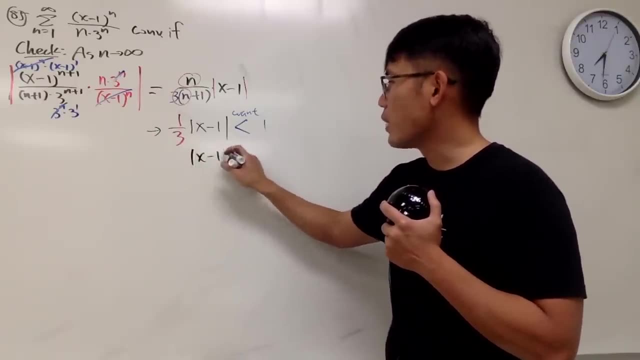 We want this to be less than 1.. And now let's just play around with this inequality. Multiply by 3 on both sides, So we get the absolute value of x minus 1 is less than 3.. And of course you can do a little bit. 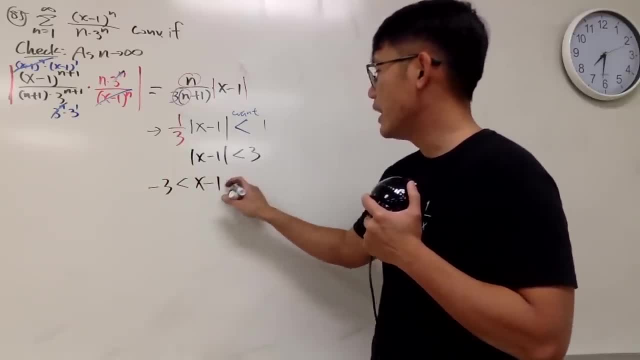 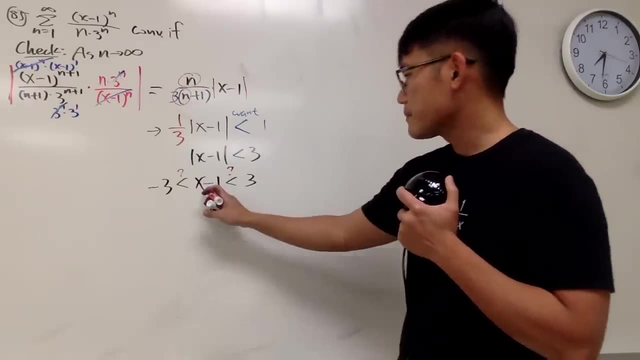 This is just x minus 1.. It's in between of negative 3 and positive 3.. And technically, I don't know the endpoints yet, I don't know what happens at the endpoints yet, And then, right here, let's just add 1 to everybody. 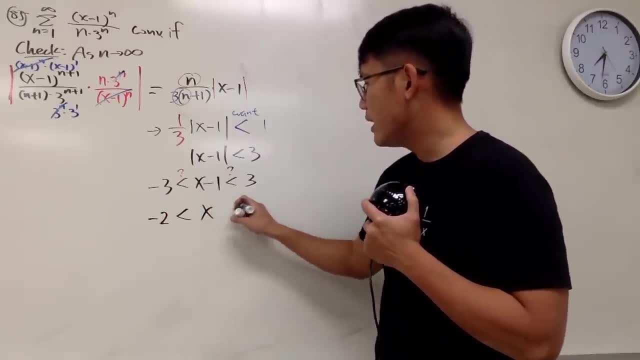 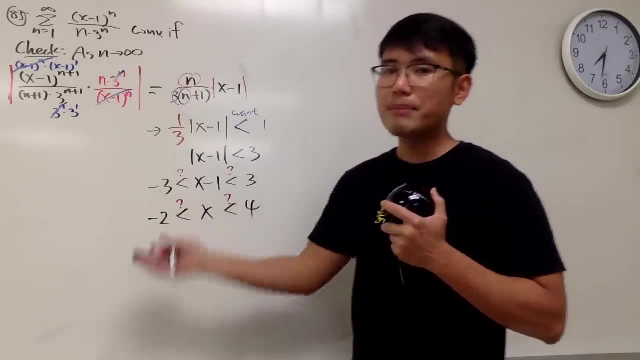 So we get negative 2. And here we have 4.. Yeah, And again I don't know. I don't know yet. So let's come back here and check. Let's check when x is negative 2.. 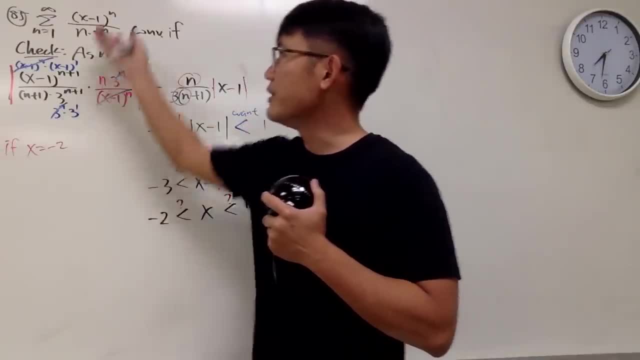 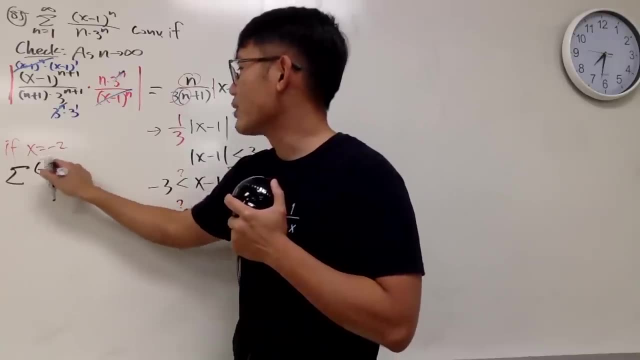 If x is negative 2, to see if this guy will converge or not. Let's look at the sum And I'm not going to write down 1 to infinity. It's too much work to write. I should have done that a long time ago, but yeah. 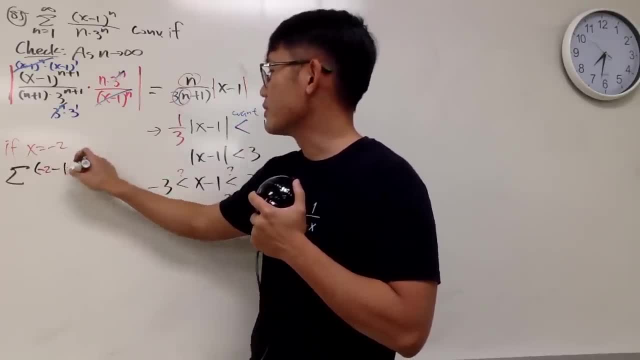 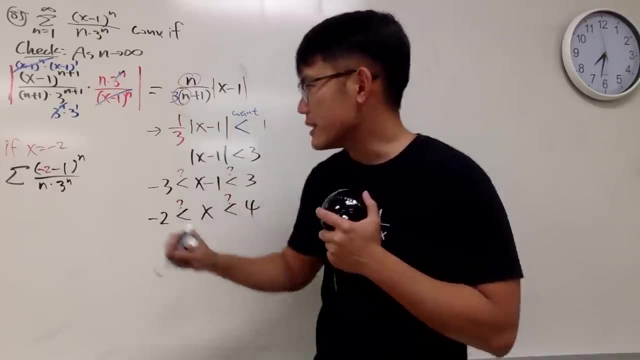 Anyway, it's this same one, So let's just do the check right here. We have n Times 3 to the n Like that. Now the good thing is: look at this right here, It's actually the sum. 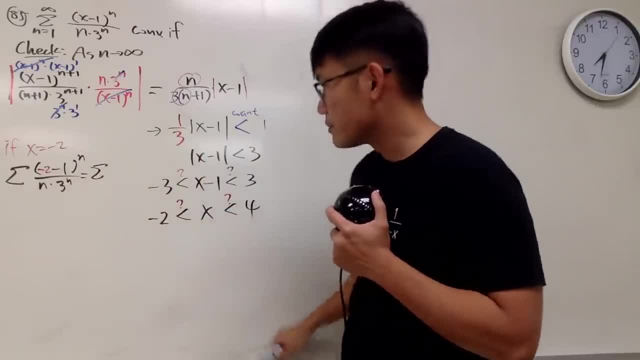 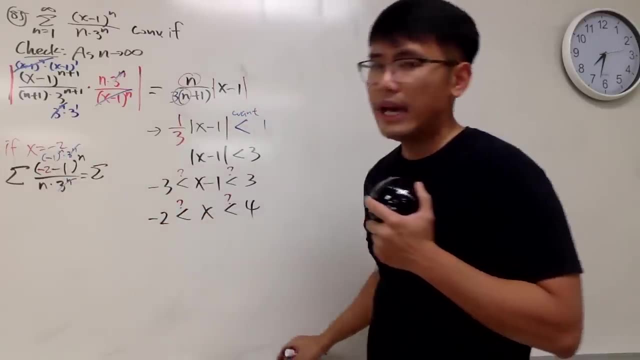 This is negative 3 to the n, Which is the same as saying negative 1 to the n times 3 to the n. So this and that will actually cancel And we end up with negative 1 to the nth power over n. 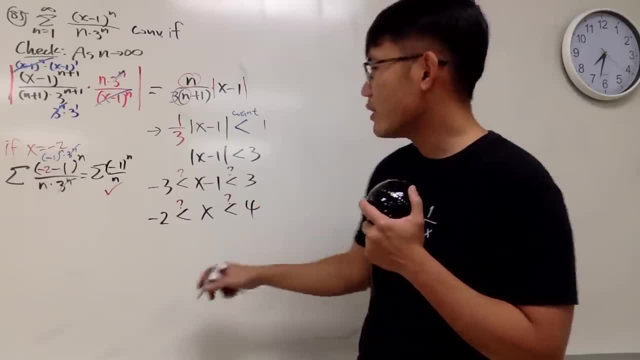 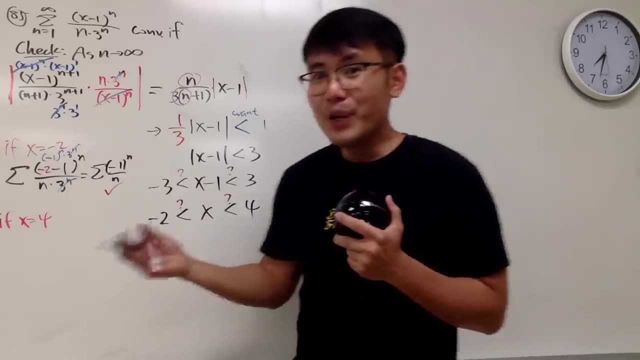 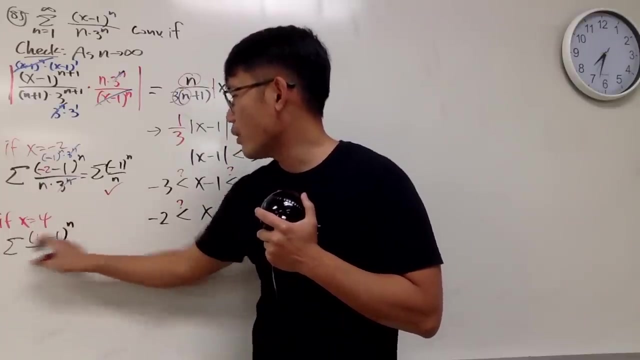 So this right here actually converges. On the other hand, though, You have 4 in there, If x is equal to 4.. We will get what? We will just get the sum as 4 minus 1 to the nth power, over n times 3 to the n. 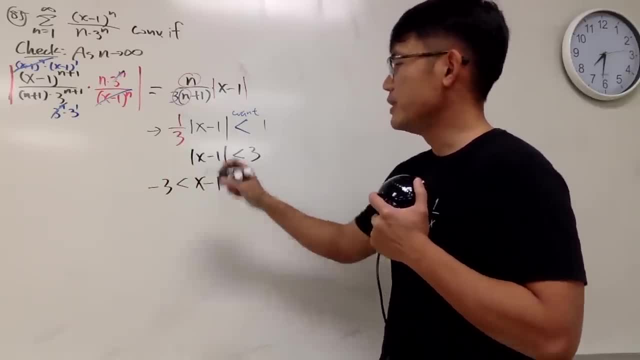 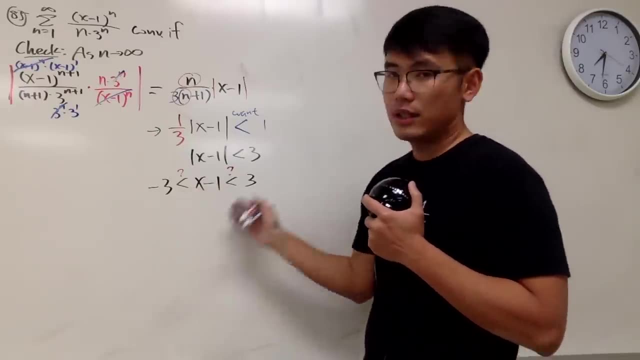 It's in between of negative 3. And pass this 3. And technically, I don't know the endpoints yet, I don't know what happens at the endpoints yet. And then, right here, let's just add 1 to everybody. 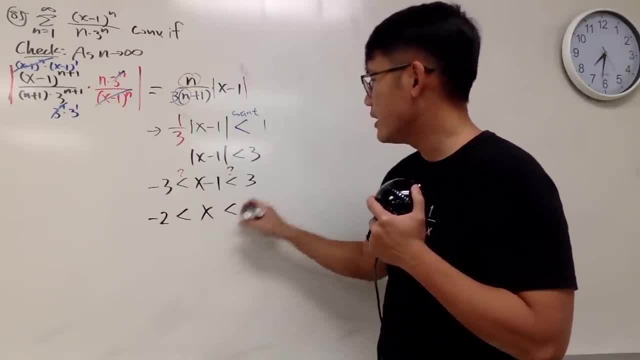 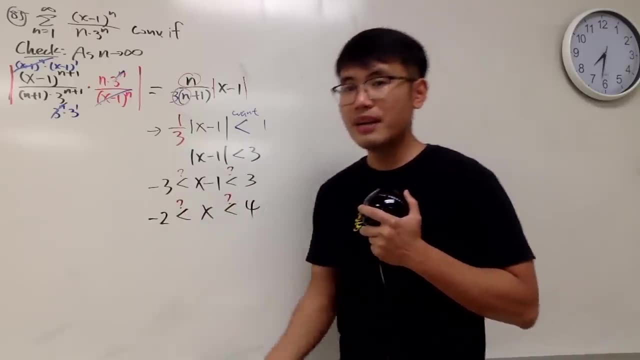 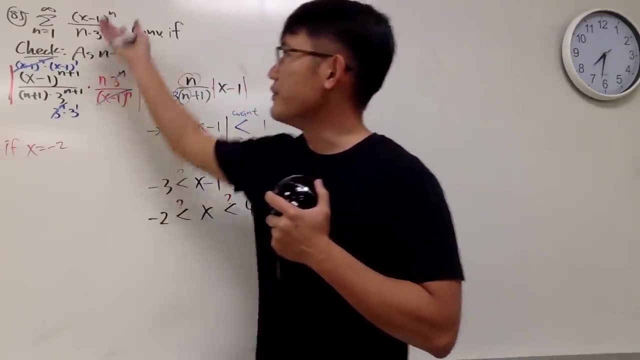 So we get negative 2.. And here we have 4.. Yeah, And again I don't know. I don't know yet. So let's come back here and check. Let's check when x is negative 2.. If x is negative 2 to see if this guy will converge or not. 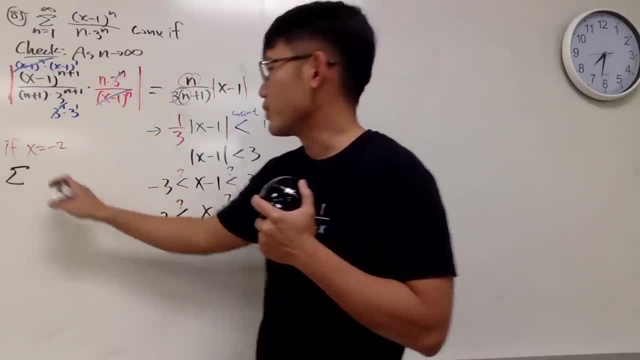 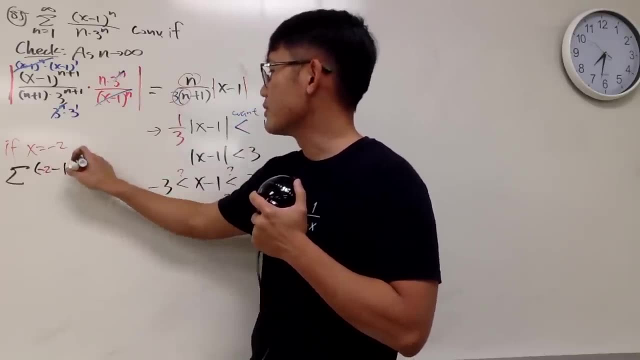 Alright, Let's look at this, at the sum, and I'm not going to write down the 1 to infinity, it's too much work to write. I should have done that a long time ago. but yeah, Anyway, it's this same one, so let's just do the check right here We have. 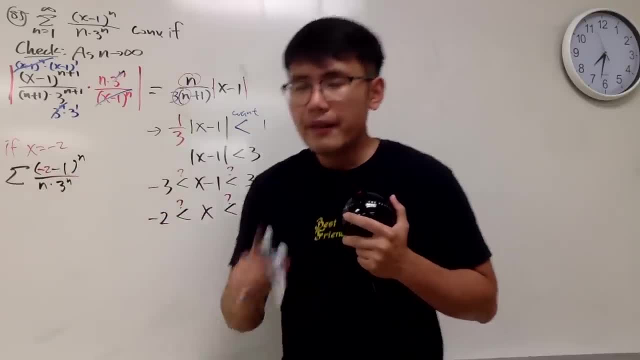 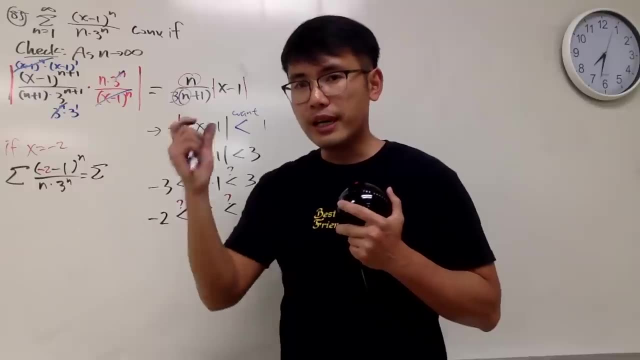 n times 3 to the n, like that. Now, the good thing is: look at this right here: it's actually the sum. This is negative 3 to the n, which is the same as saying negative 1 to the n. 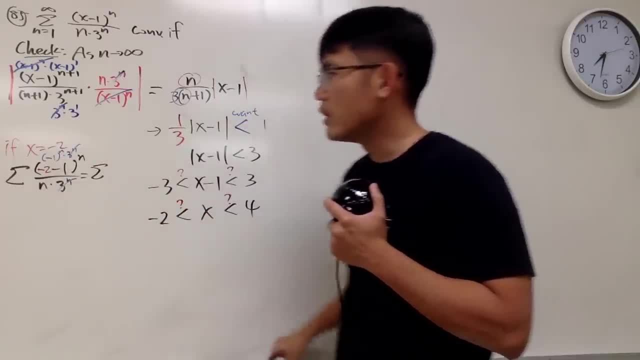 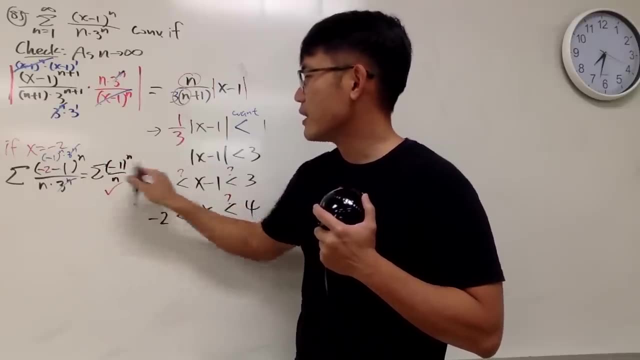 times 3 to the n. so this and that will actually cancel, and we end up with negative 1 to the nth power over n. so this, right here, actually converges. On the other hand, though, if you have 4 in there, 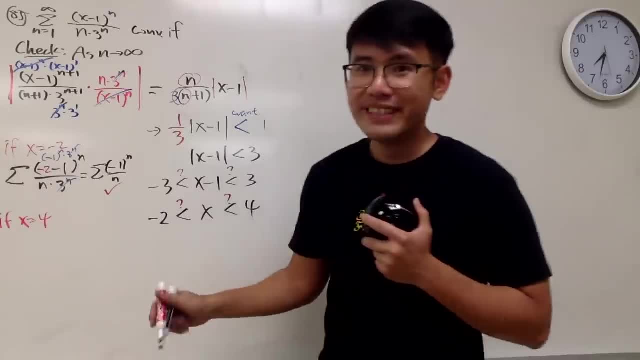 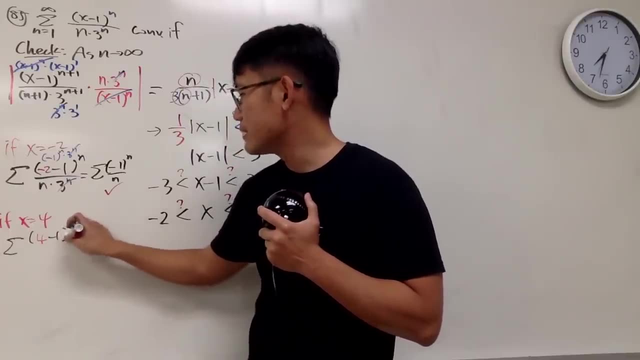 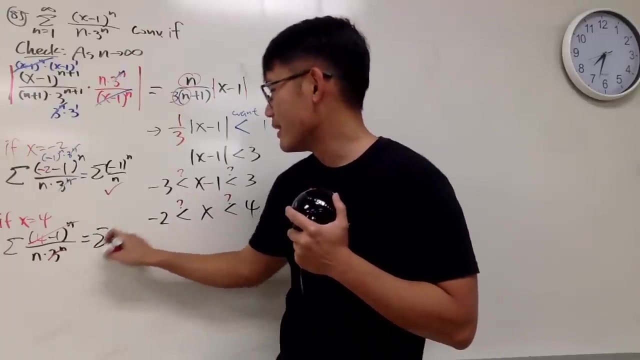 if x is equal to 4, we will get what? We will just get the sum as 4 minus 1 to the nth, power over n times 3 to the n, And that cancels out. You just get the sum as 1 over n, like this: 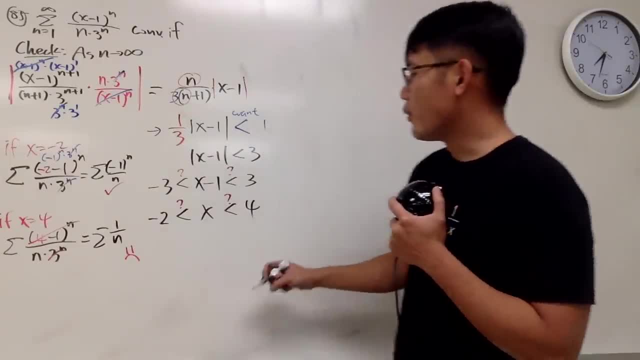 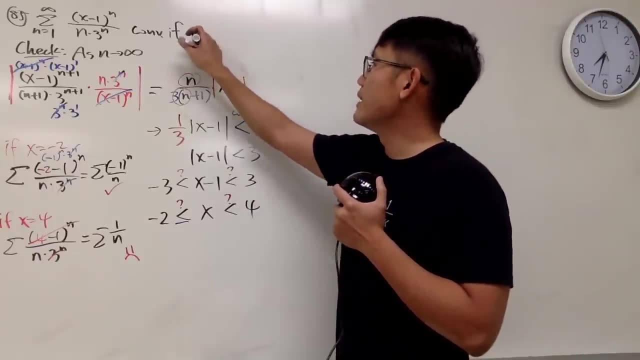 So diverges. Therefore, I want to include the negative right here, but not that, So this converges if we have x in between of negative 2, including that and less than 4, not including the 4.. 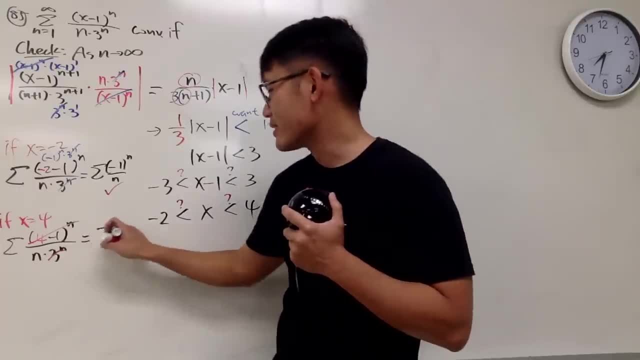 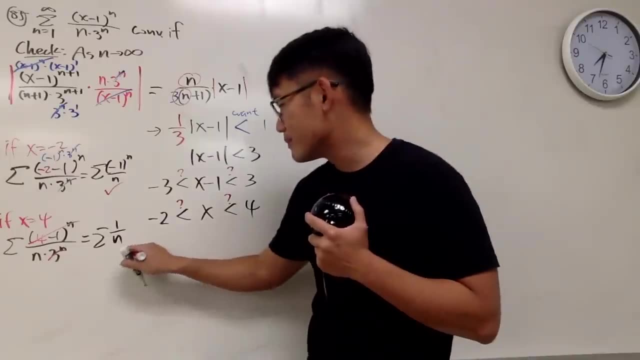 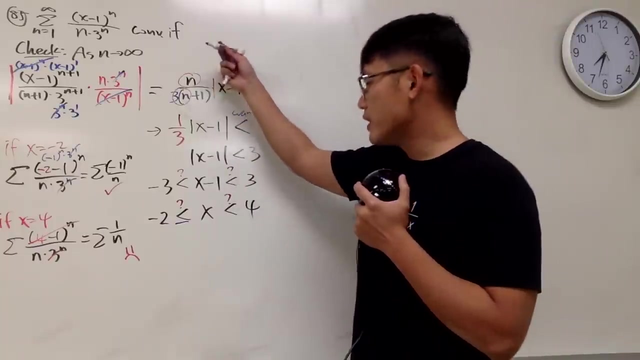 This and that, cancel out. You just get the sum as 1 over n, Like this, So diverges. Therefore I want to include the negative right here, But not that. So this converges If we have x in between of negative 2.. 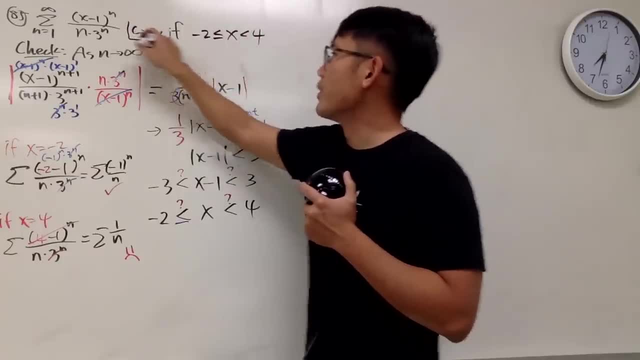 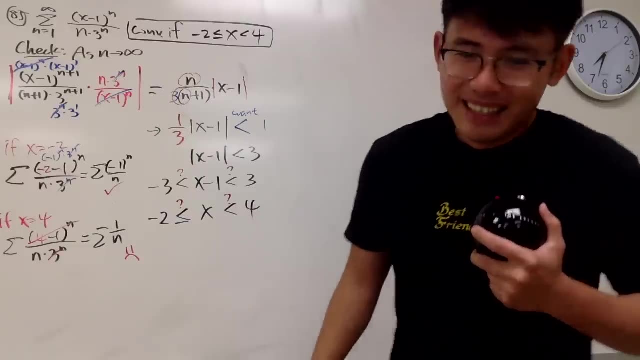 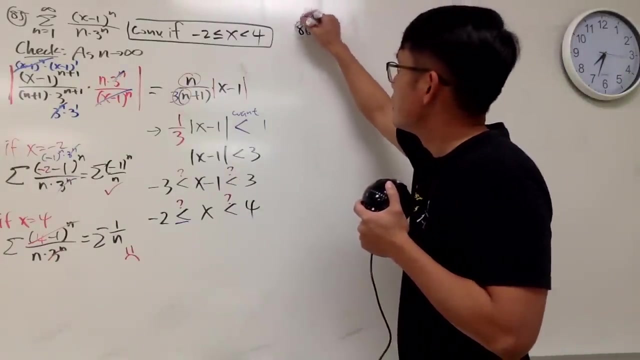 Including that, And less than 4.. Not including the 4.. So that's what we have. Okay, 15 questions, Oh my god. Okay, Now 86.. The sum as n goes from I put down 1- to infinity. 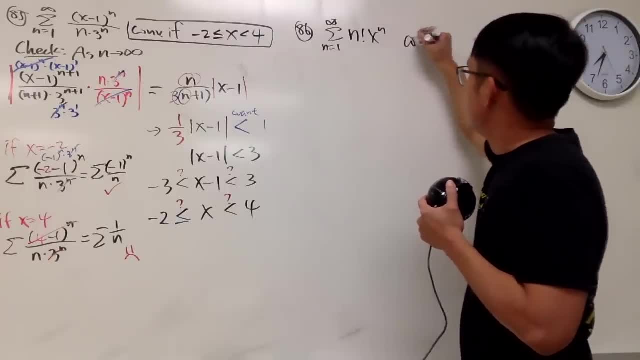 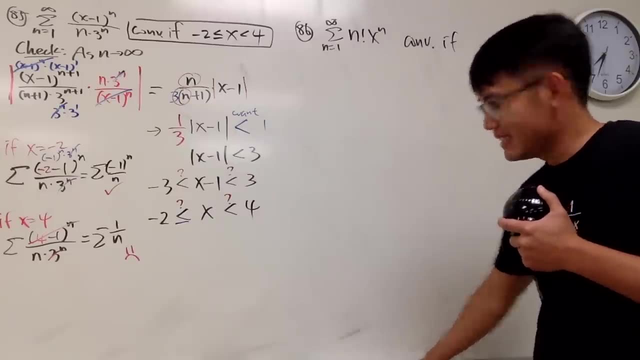 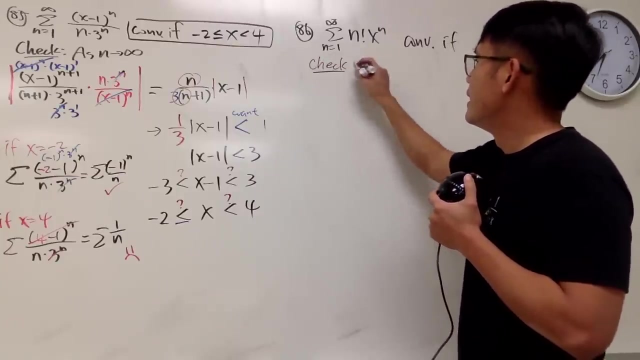 And factorial x to the n Converges. If what? Now Let's just do the ratio test, Why not? Alright, So go ahead and check As n goes to infinity. Alright, So ratio test in action. 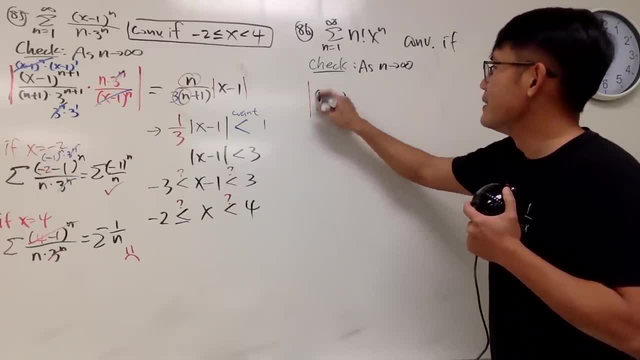 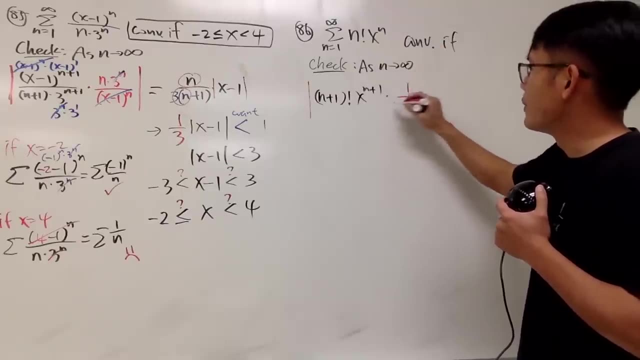 Here Put down the absolute value N plus 1.. Factorial that X to the n plus 1. Right, And You multiply by the reciprocal, Namely You put 1 over n. factorial X to the n. 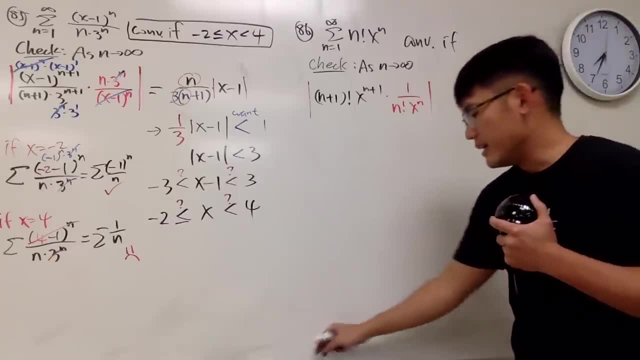 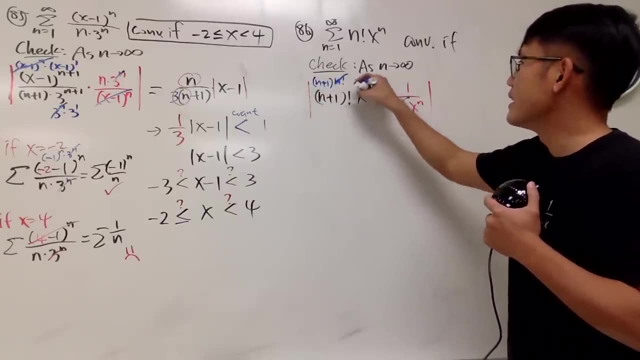 Like this. Okay, So Again, This right here Is N plus 1. Times n factorial: This and that cancel. This is x to the n times x This and that cancel. Therefore, All in all, We end up with: 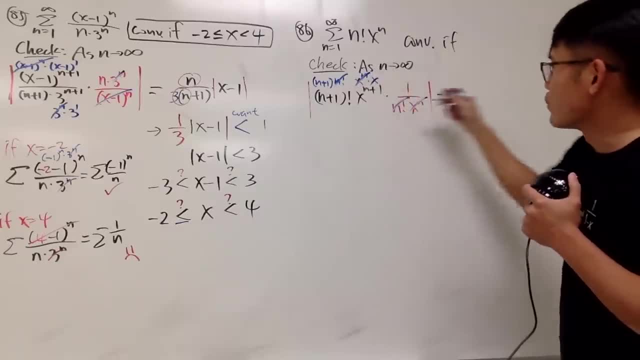 N plus 1 can be come out right here: N plus 1.. But we have to multiply this right here, So We end up with N plus 1.. But we have to multiply this with The absolute value Of x. 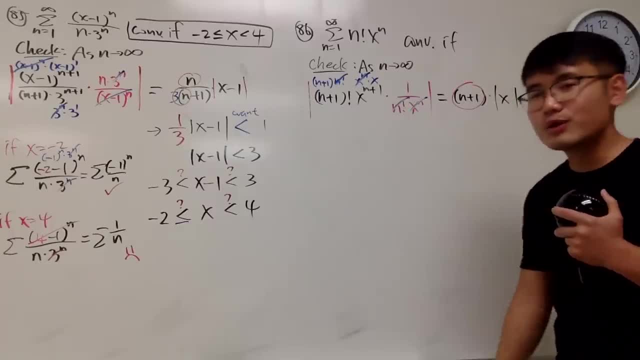 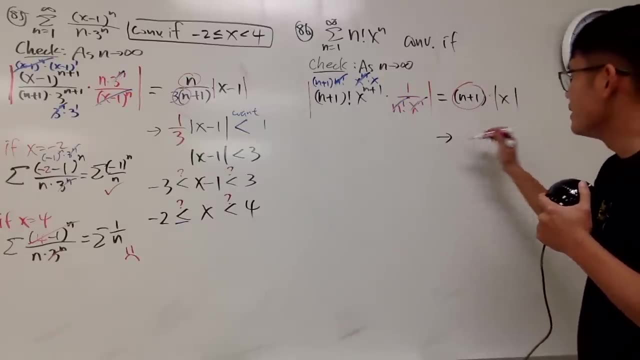 And you know the deal. Take this, As n goes to infinity, But this time N plus 1. Also Go to infinity as well. This is going to be Infinity Times, the Parenthesis Times, the absolute value of x. 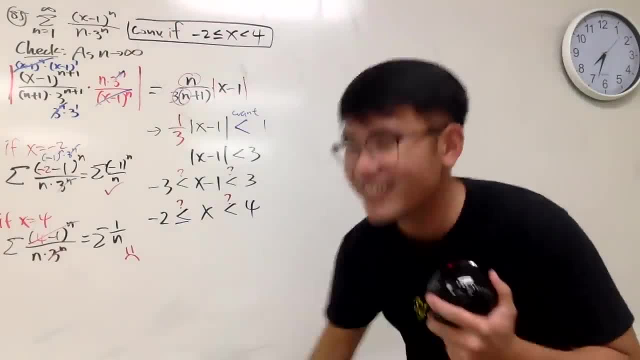 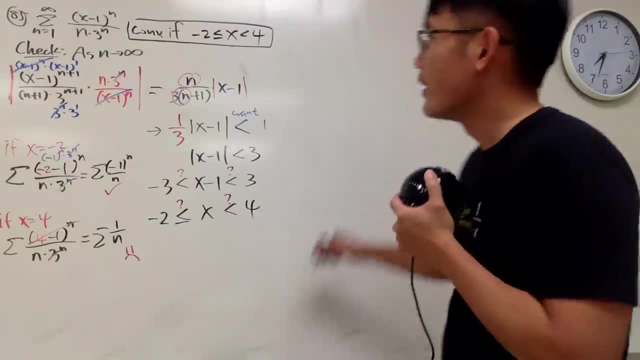 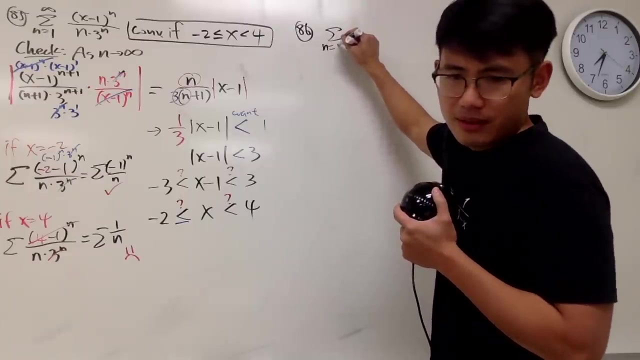 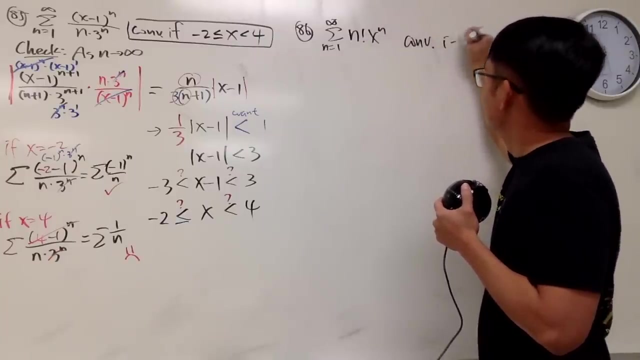 So that's what we have. Okay, 15 questions, Thanks, Oh my god. Okay, Now 86.. The sum as n goes from I put down 1 to infinity n, factorial x to the n converges, if what. 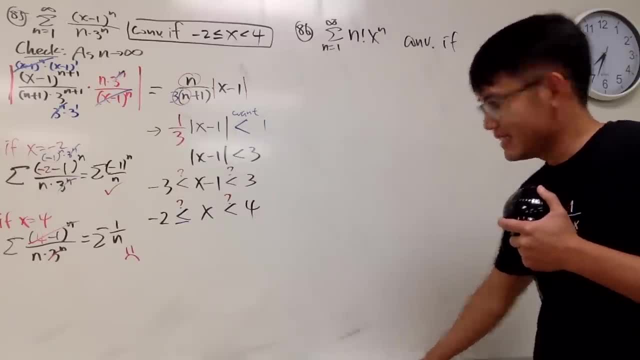 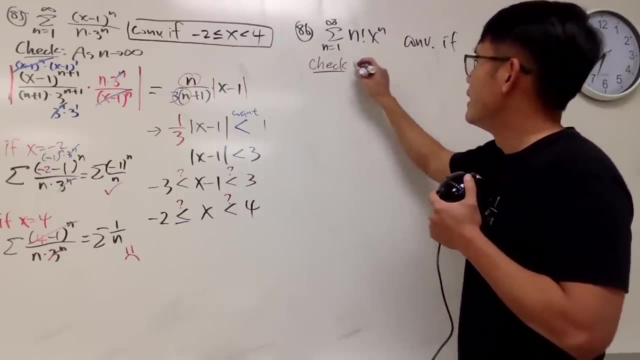 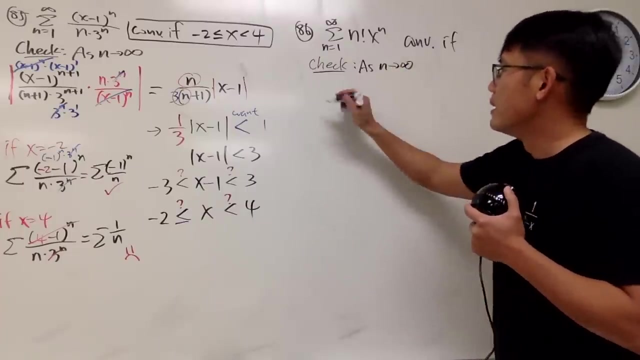 Now let's just do the ratio test, why not? Alright, so go ahead and check. S: n goes to infinity, alright. So ratio test in action Here. put down the absolute value n plus 1, factorial, that x to the n plus 1, right. 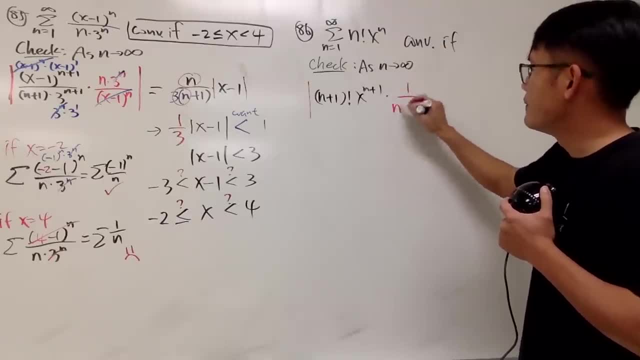 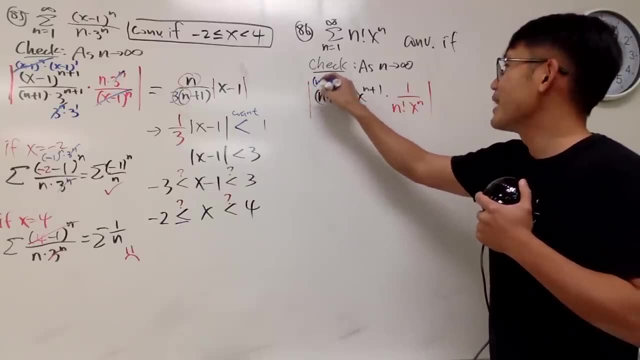 And you multiply by the reciprocal, namely you put 1 over n factorial, x to the n, like this: Okay, so again, this right here is n plus 1 times n factorial. this end up cancel. So this is x to the n times x. 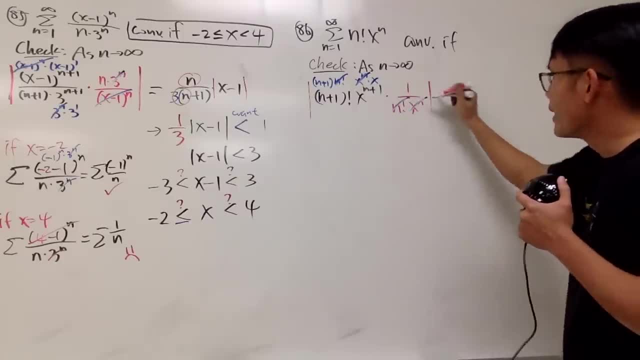 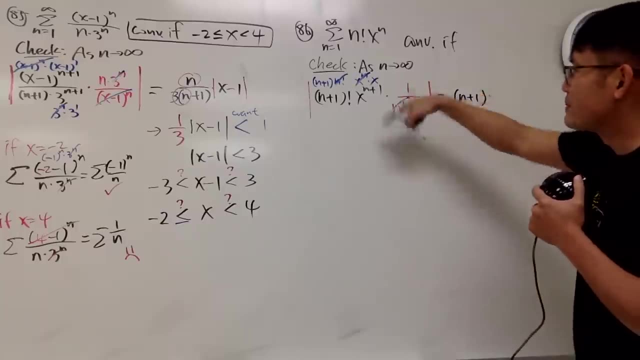 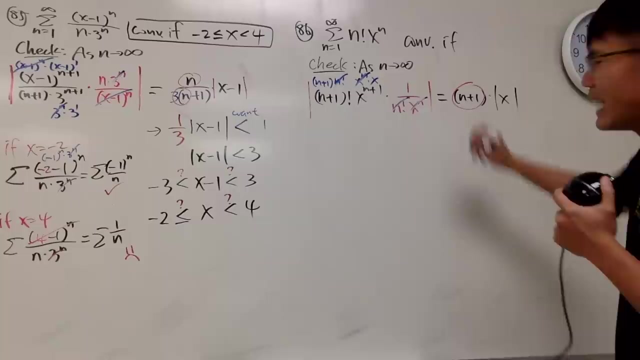 this and that cancel. therefore, all in all, we end up with n plus 1 can be come out right here: n plus 1, but we have to multiply this with the absolute value of x and you know the deal. take this, as n goes to infinity, but this time n plus 1 also go to infinity as well. 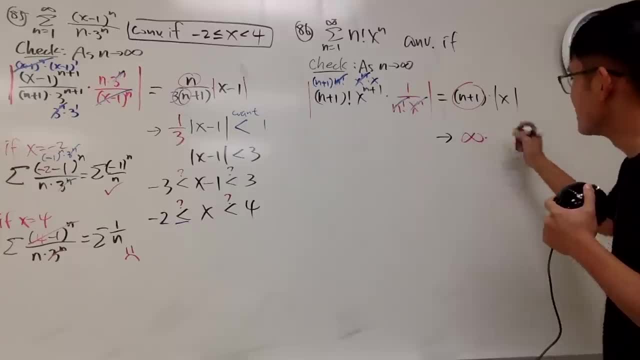 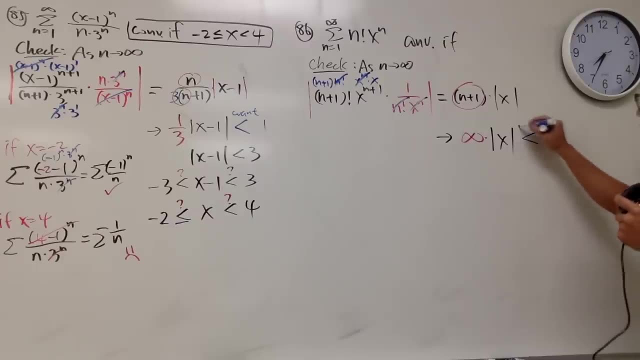 so this is going to be infinity times the parenthesis times, the absolute value of x. and now, right here, we want to have this to be less than 1, how is this even possible? right this, right here. some of you guys are going to be like mad. 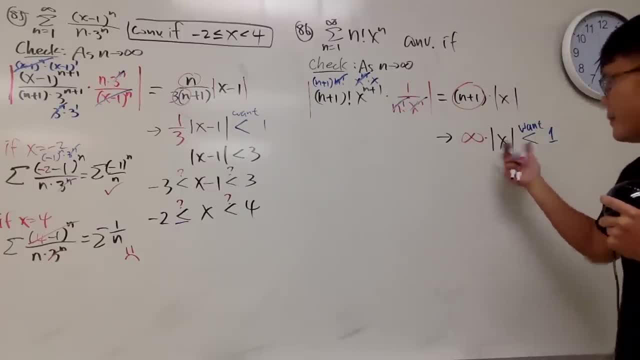 but here is the only case. this is the situation. I'm not going to divide both sides by infinity whatsoever. I'm not going to do that and I'm not going to tell you infinity times the absolute value of 0 is less than 1,. 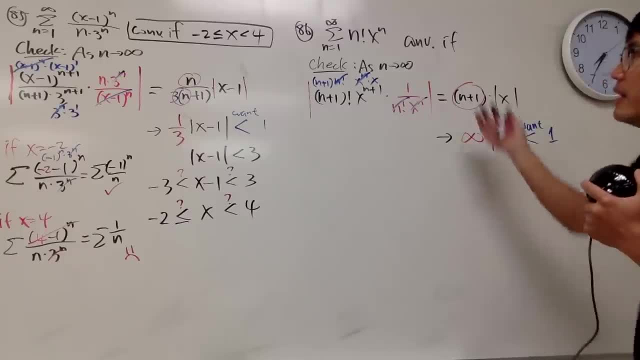 I'm not going to tell you, I'll just tell you. when this kind of things happen in the power series situation like this, I'll just say true, I'll say only true, I'll just say, I'll just say only if x is equal to 0, because what matters? 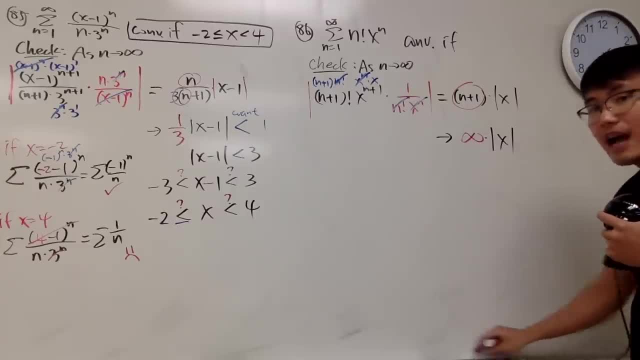 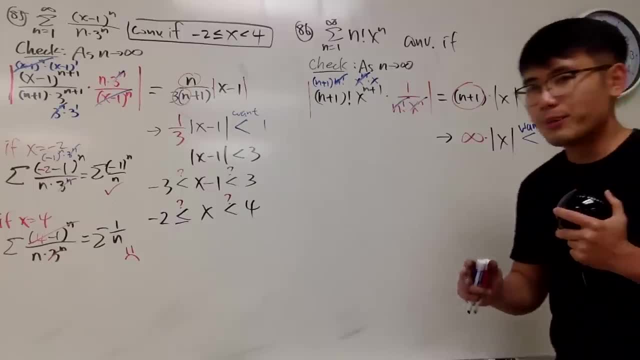 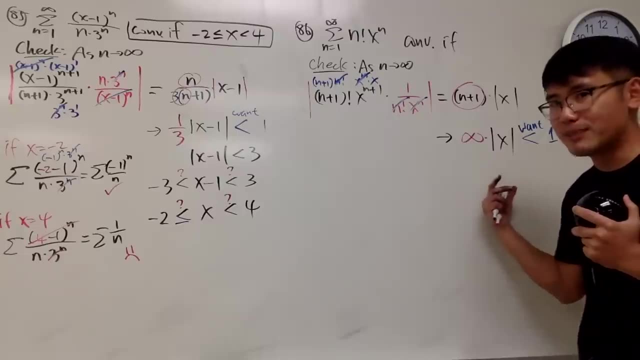 Even possible. Right This, right here. Some of you guys Are going to be like Mad, But Here is the only Case. This is The situation. I'm not going to divide both sides By infinity Or whatsoever. 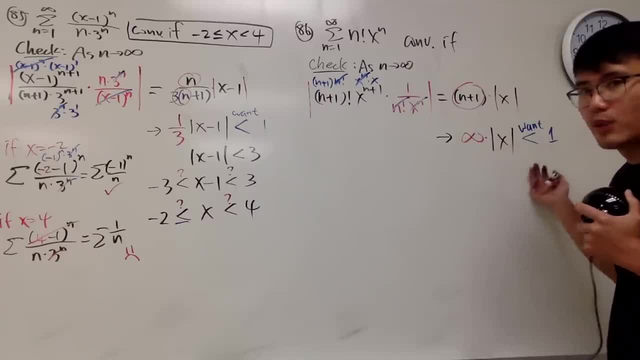 I'm not going to do that And I'm not going to tell you Infinity times The absolute value of 0. Is less than 1.. I'm not going to tell you. I will just tell you When this kind of things happen. 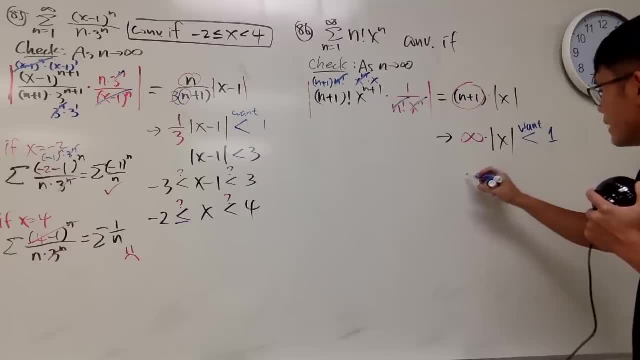 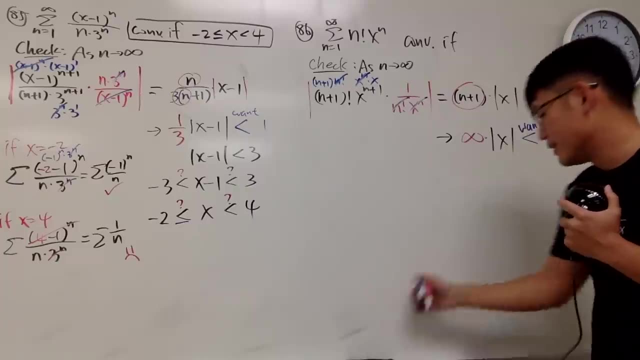 In the power series situation Like this: Um, I will just say True, I will only. I will say only. I will just say I'll just say Um, Only if X is equal to 0. Because 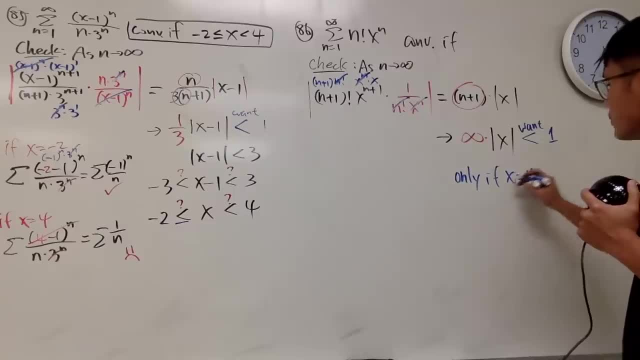 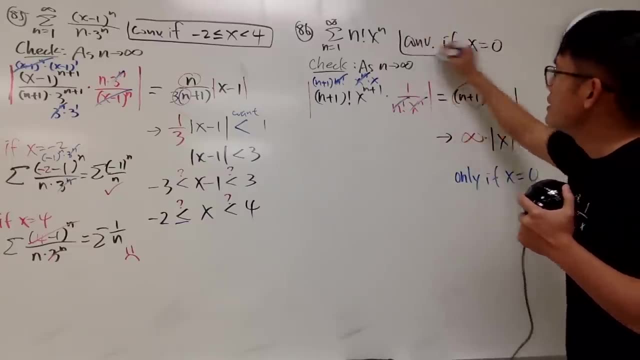 Water matters When you say This right here: converges If X is Equal to 0. And this is the only number That will make this work. The idea is that You technically Put 0 right here First. 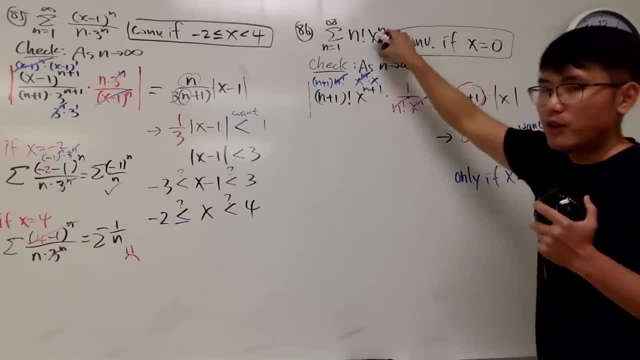 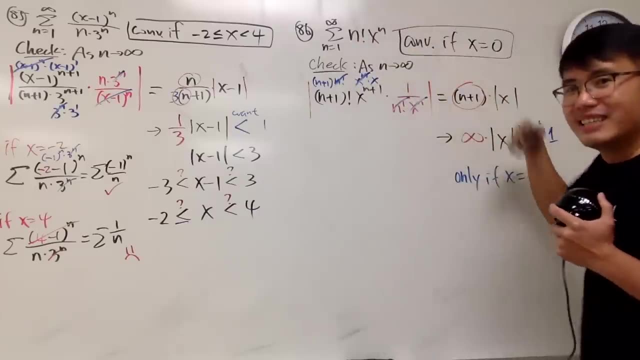 And you work that out And you don't do anything Like Crazy. This is just a bunch of like Adding 0's. So This right here Is The only Thing. So This right here Is just. 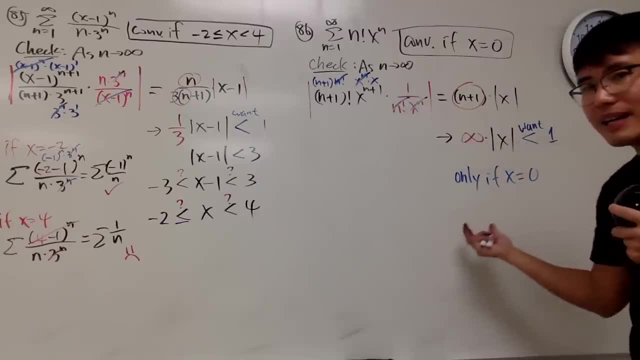 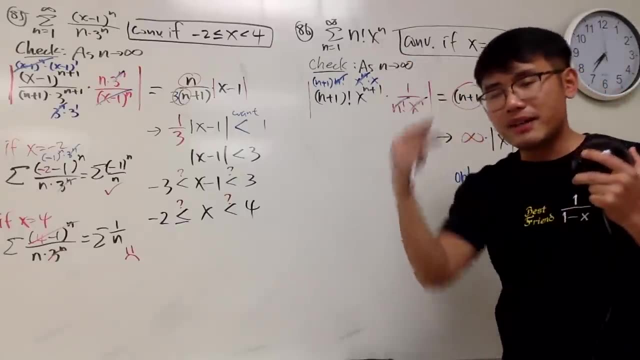 I know It sounds kind of bizarre Because you end up with An infinity times 0. But again, When this happens, Just remember X has to be 0.. To make this true, Sometimes You may have X minus 5.. 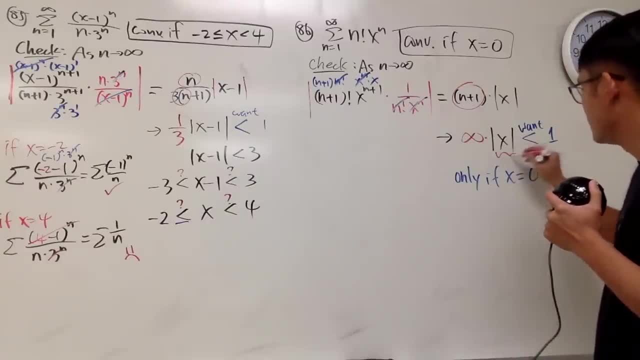 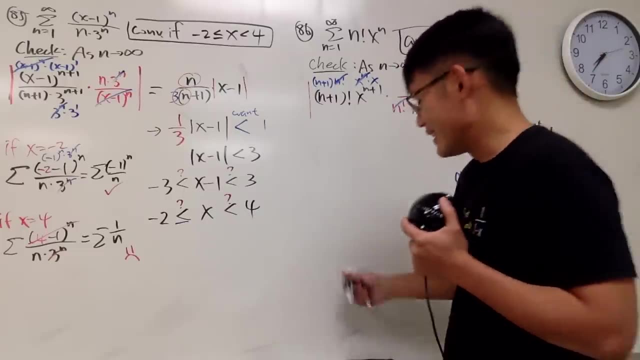 And a 2 nth power. In that case X will be 5. So that you can produce 0. So You want This To be That Right, So Hopefully That's a. I will make another video. 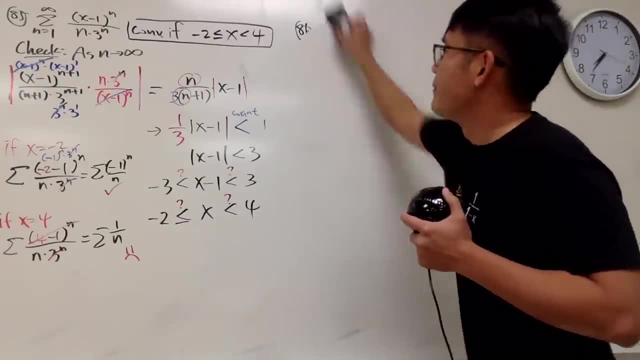 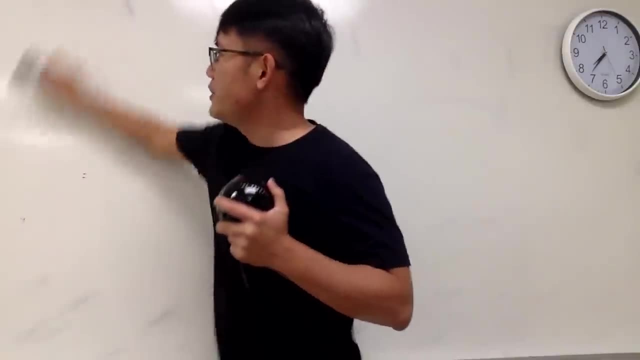 Not 100 of them. Oh So, If you guys can Seriously Help me To share this video With your Students, Your Classmates, Your Teachers, Your Professors, If you are Cats, 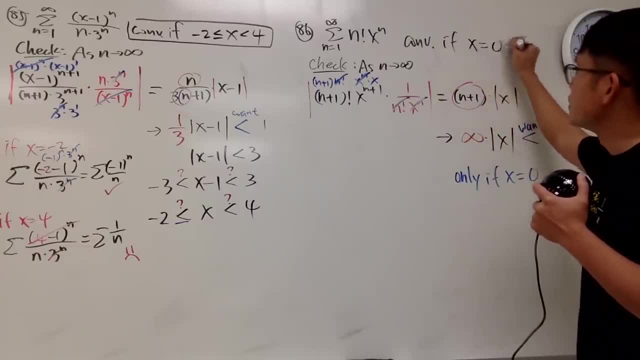 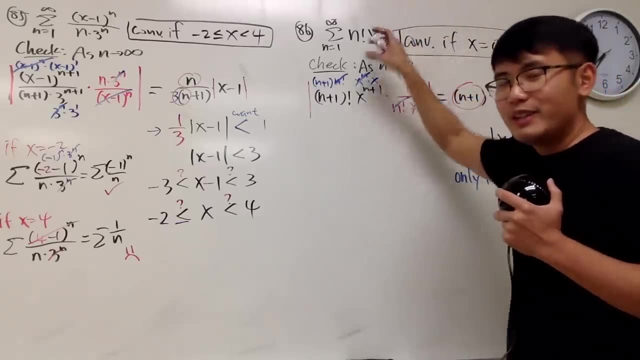 when you say this right here: converges if x is equal to 0, and this is the only number that will make this work. the idea is that you technically put 0 right here first and you work that out and you don't do anything like crazy. this is just a bunch of like adding 0s. 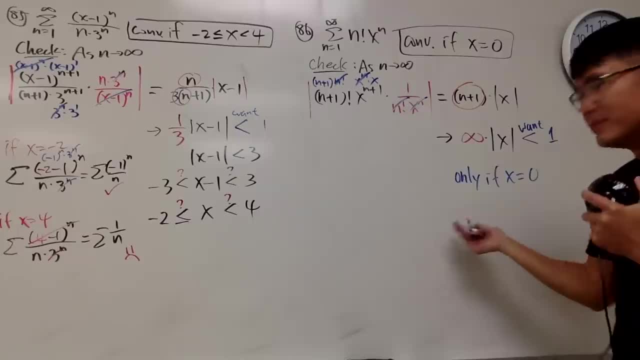 so this right here is just. I know it sounds kind of bizarre because you end up with an infinity times 0, but again, when this happens, just remember x has to be 0. to make this true, sometimes you may have x minus 5 and 2n power. 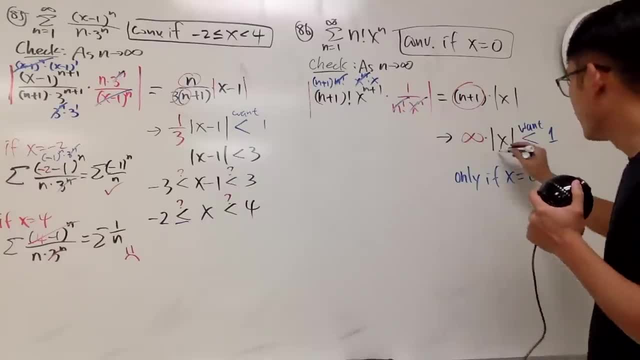 in that case, it's going to be 0, and you're going to have x minus 5, and you're going to have x minus 5, and x would be 5, so that you can produce 0,. so you want this to be that right. 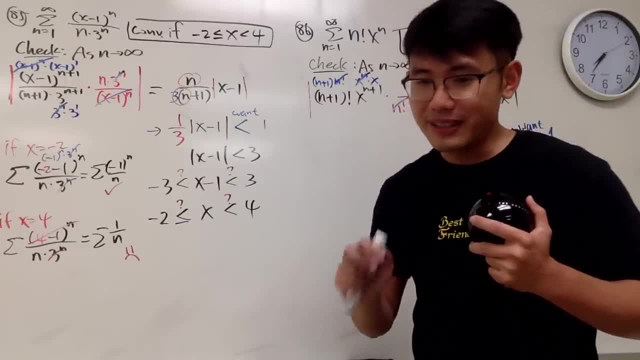 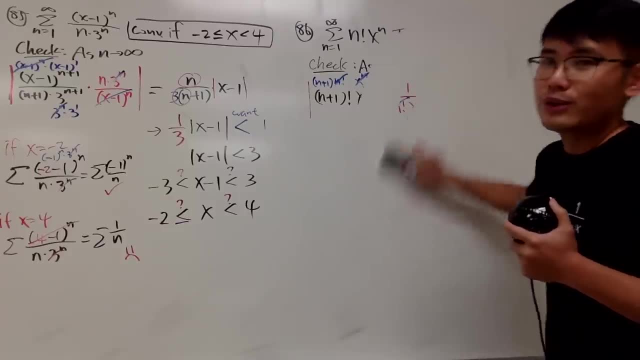 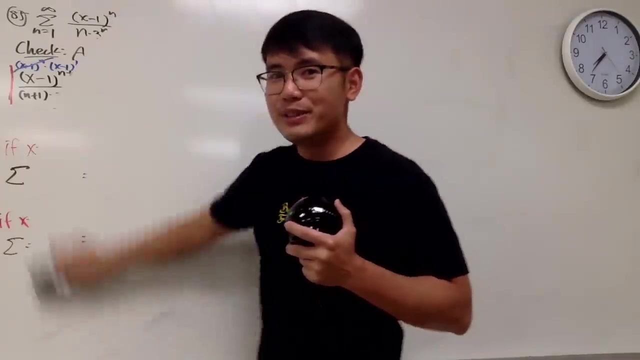 So hopefully that's a good enough explanation, right? If you guys are not happy with it, I will make another video, not 100 of them. So if you guys can seriously help me to share this video with your students, 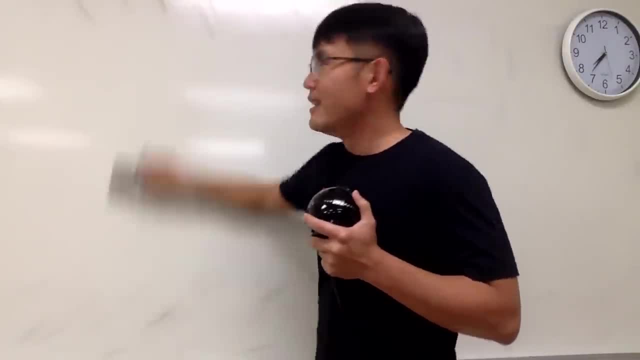 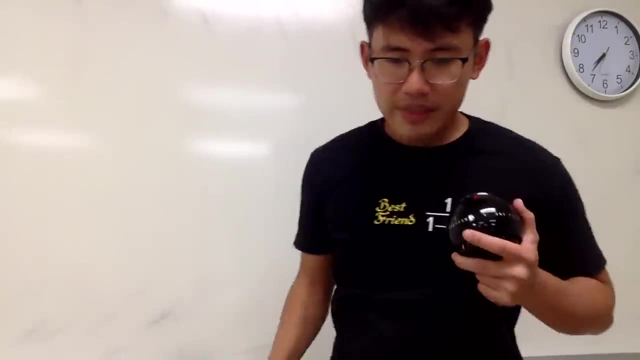 your classmates, your teachers, your professors. if you guys can help me to share this video, if you guys can help me to share this video with your cats- they also like calculus. share with them as well. Now, crazy, crazy, crazy number 87,. how did I come up with all these crazy equations? 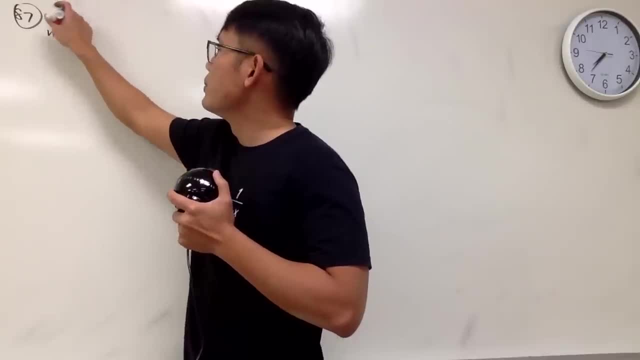 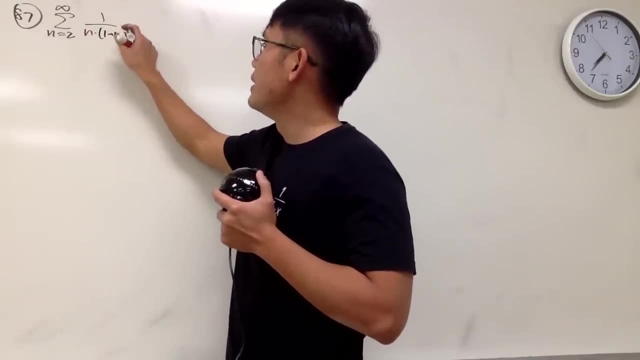 Hmm, the sum as n goes from 2 to infinity and we have 1 over n times ln, n raised to the kth power. I don't like to use x in the power, so that's why I use k. So this right here. 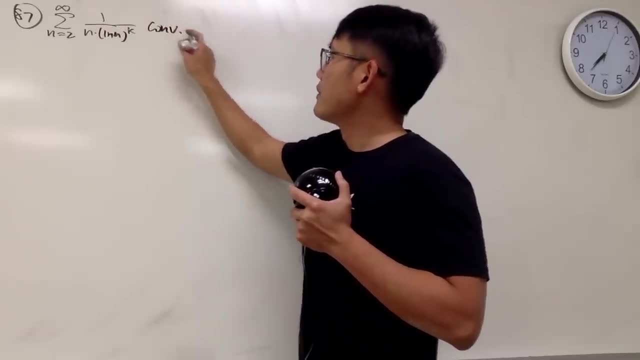 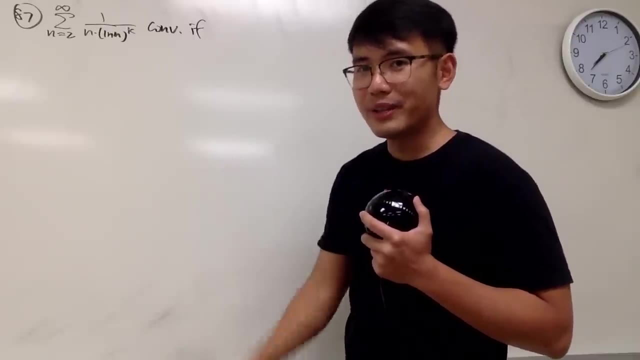 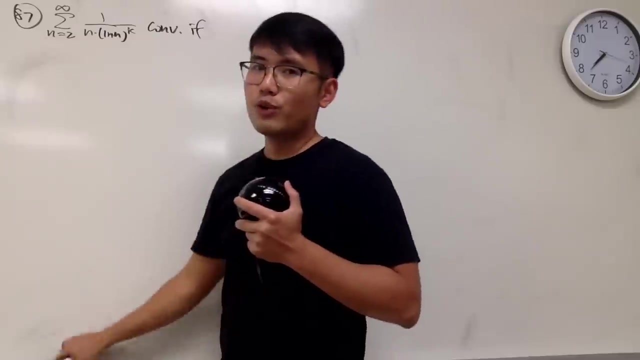 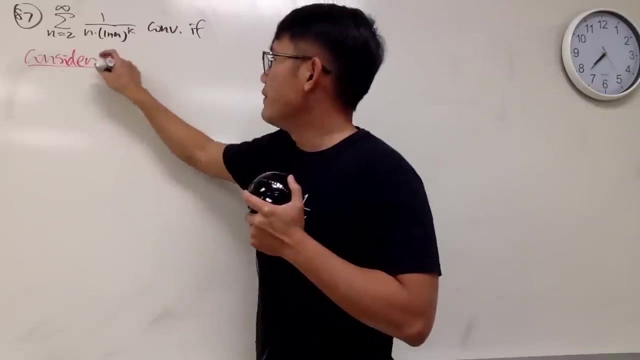 converge. if k is what right Now to do this one, we'll take this and change that to the integral case. So I'll just say: oh man, I didn't just follow my same format. I will say: consider: still in red, f of x, still 1 over x, right, and then parentheses: ln, x. 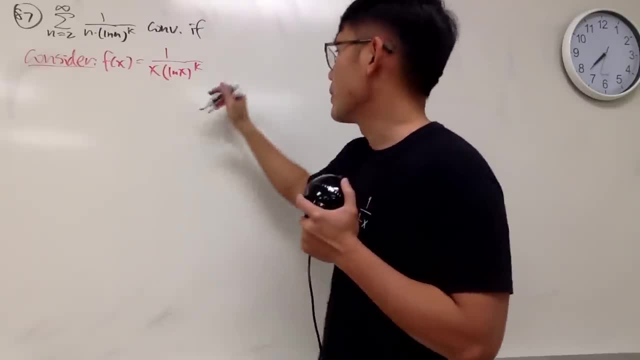 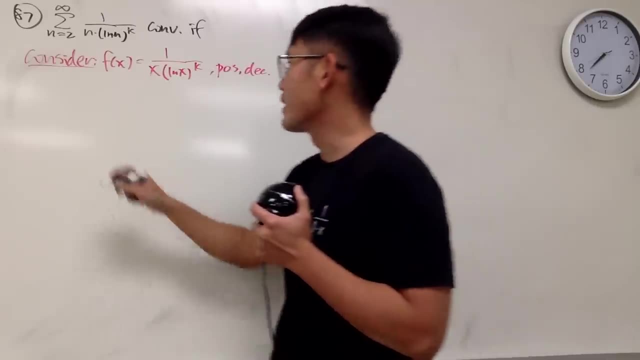 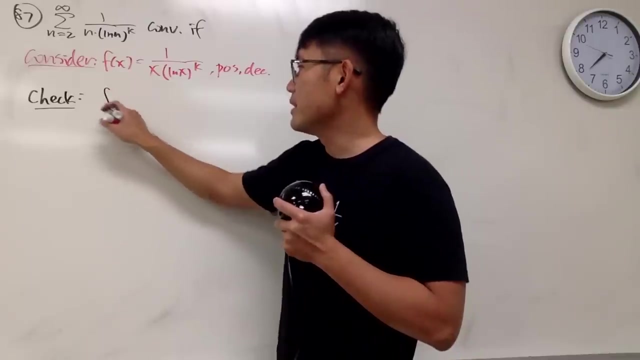 to the kth power. Well, let's just check. well, let's do it again: Positive decreasing, draw the picture seriously up to you, okay. And we just want to check right. We check the limit. well, not limit the integral from 2 to infinity. 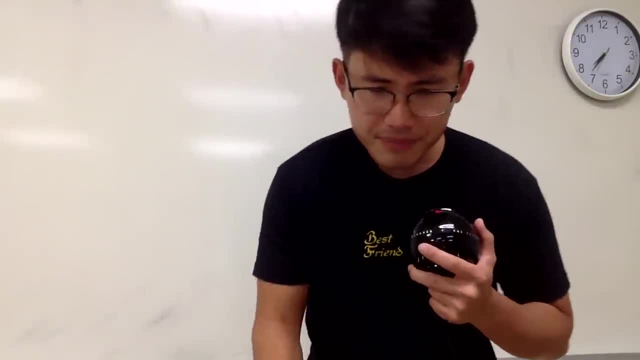 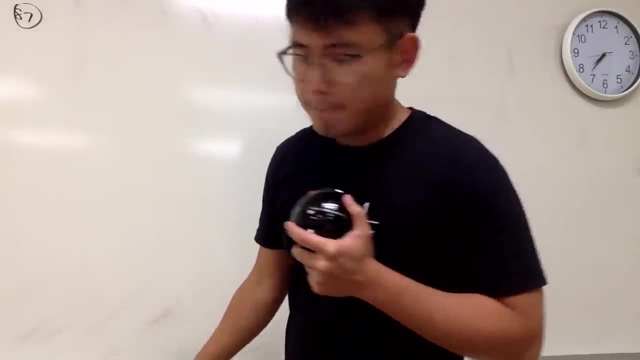 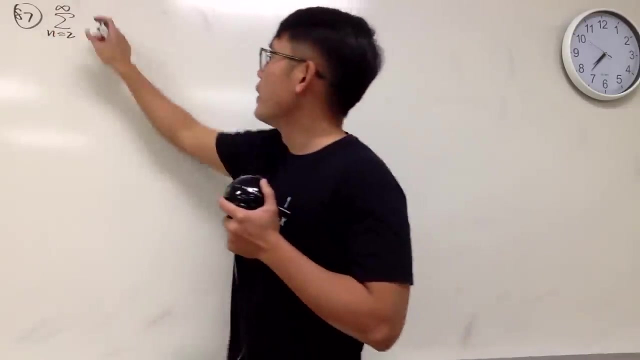 They also like Calculus. Share with them As Well. Now, Crazy, Crazy, Crazy Number 87.. The Sum As N Goes From 2. To Infinity, And We. 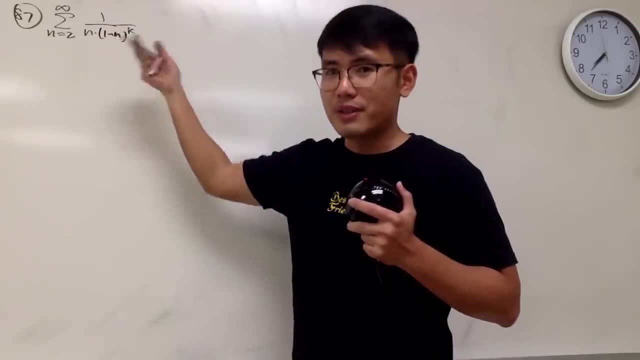 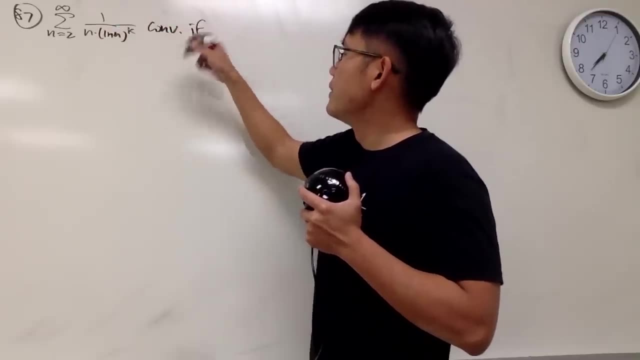 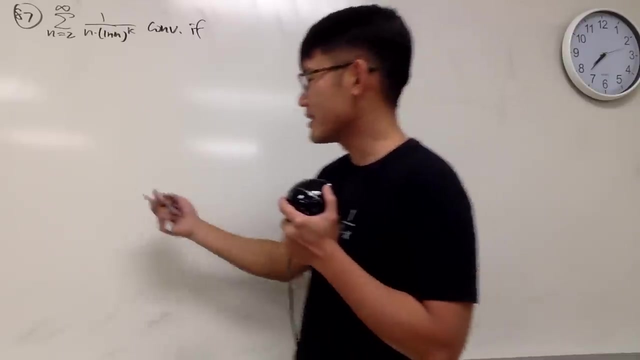 Have: 1. Over N Times L N N Raised To The Case Power I Don't Like To Use, So Just Say: Oh, Man Doesn't. 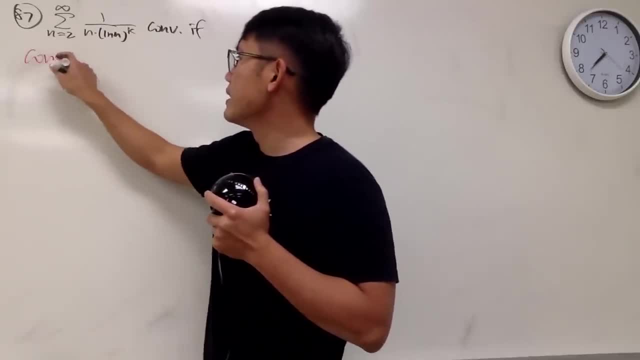 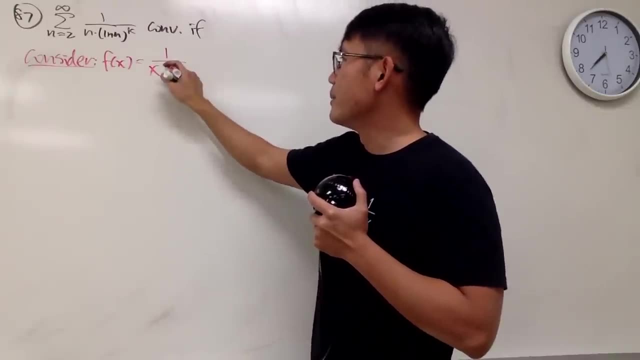 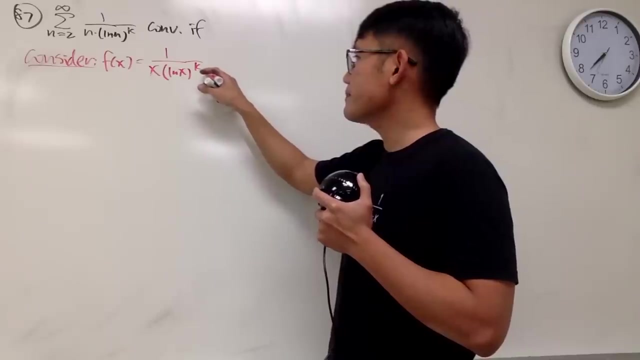 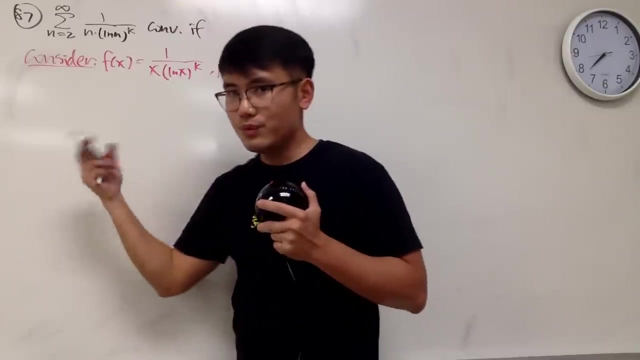 Just Still Follow My Same Format. I Will Say: Consider: Still In Red F Of X, Still 1. Over X Right. And Then We Just 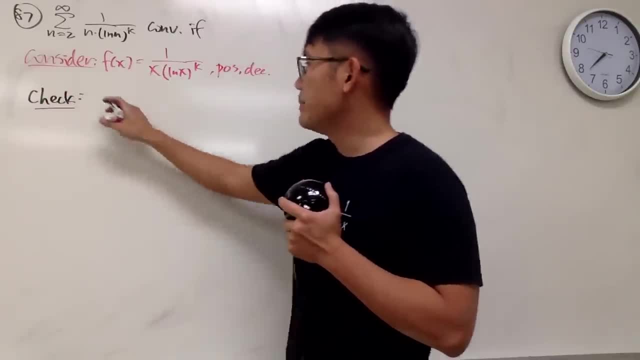 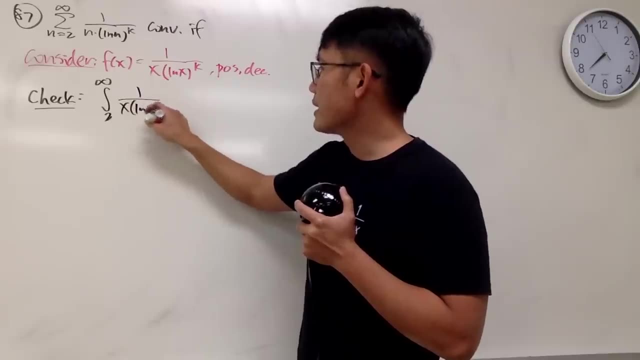 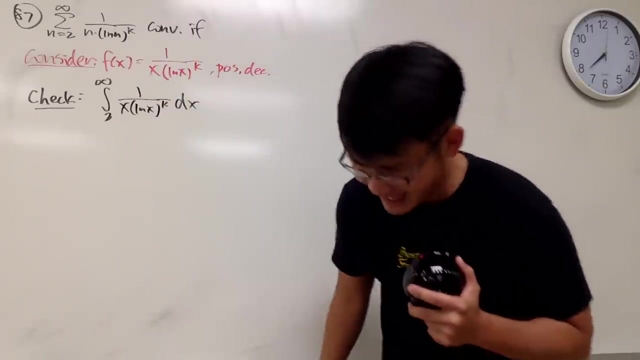 Want To Check The Limit Or Not Limit The Integral From: 2. To Infinity. 1. Over X Parentheses, L, N, X To The Case. 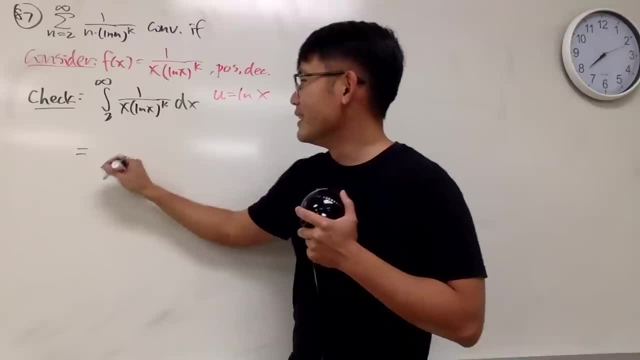 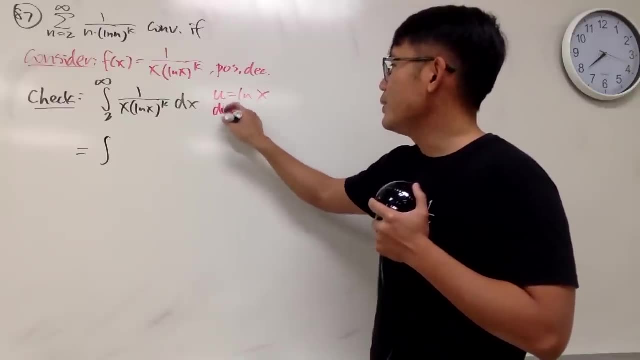 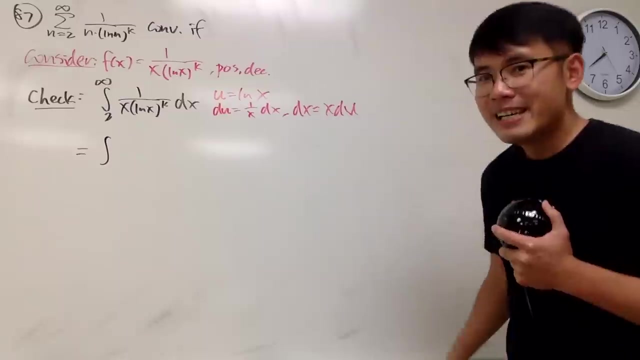 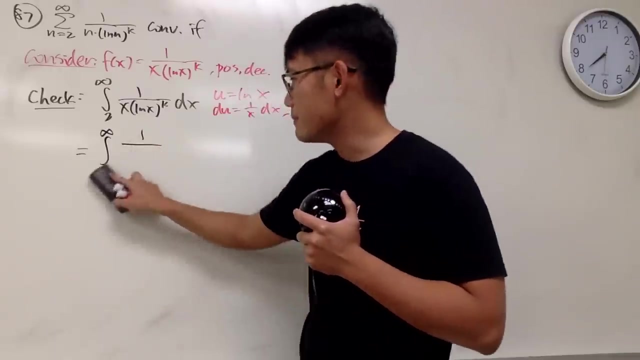 Power, X To Infinity. But This Right Here Is Equal To The Integral Of D? U Is Equal To: 1. Over X, D, X And. 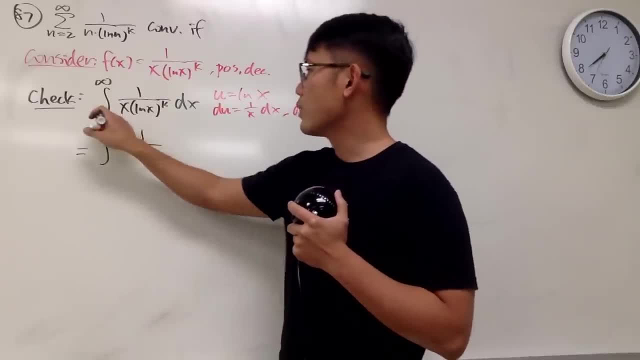 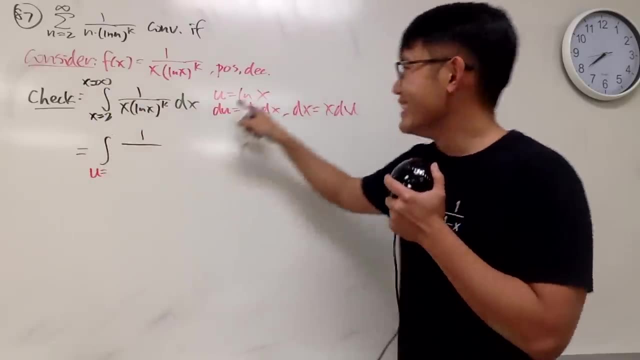 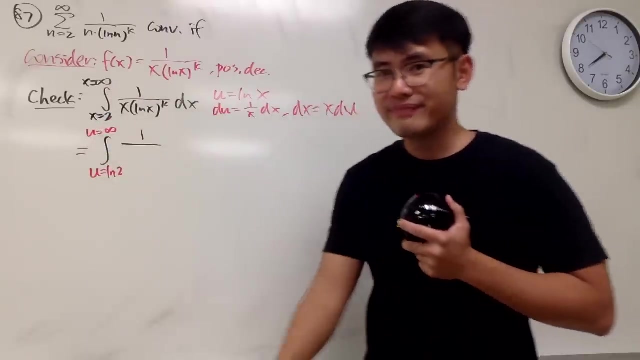 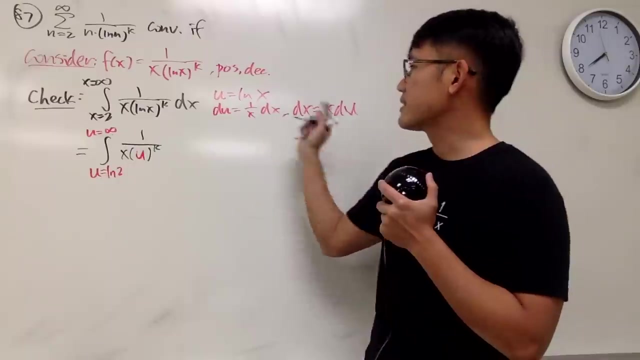 D? X Is The Same As X. D? U Will Go When You Plug In 2.. Into Here You Get U Is L N, 2.. 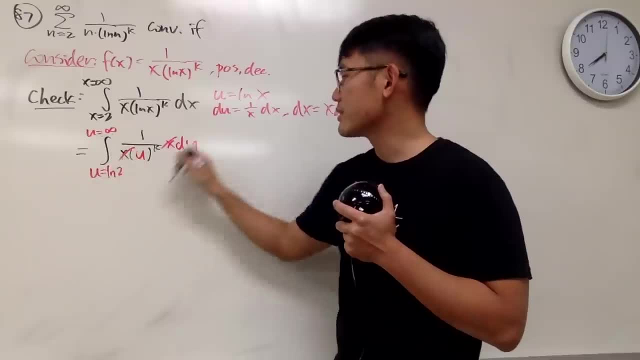 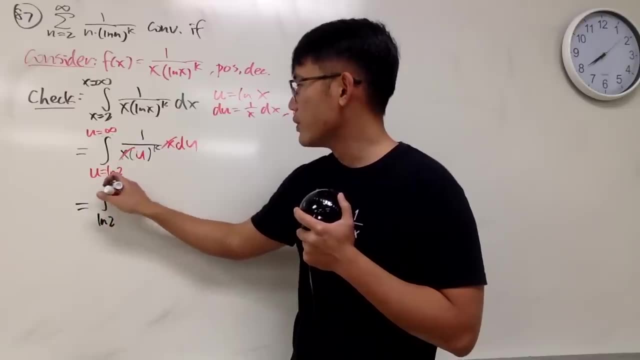 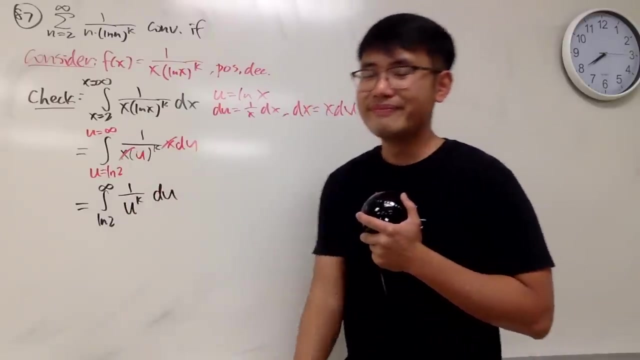 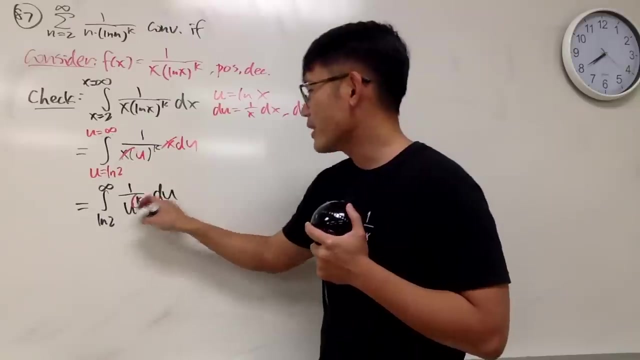 Plug In Infinity, Here U Will Be Infinity, And Then Here We Have Actually 1. Over U To The Case. Power D U. Yes, We. 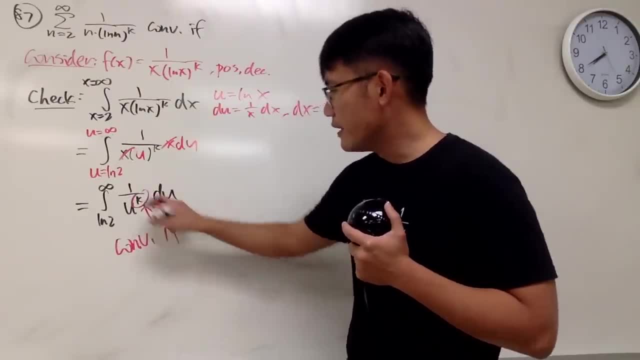 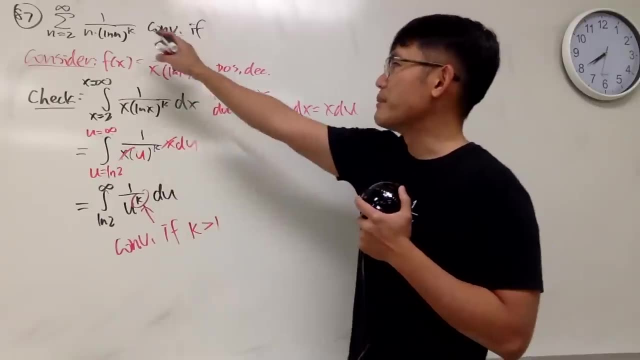 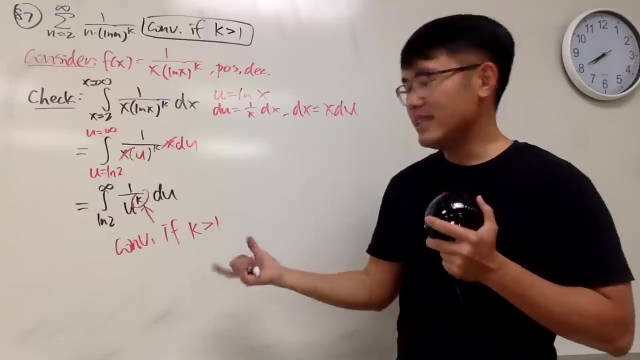 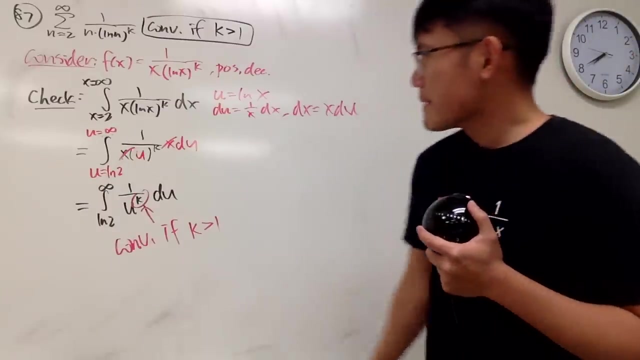 Have Talked About This Before. This Is The P Integral, The P Test For The Integral. So If You Know Something Like These Things, You 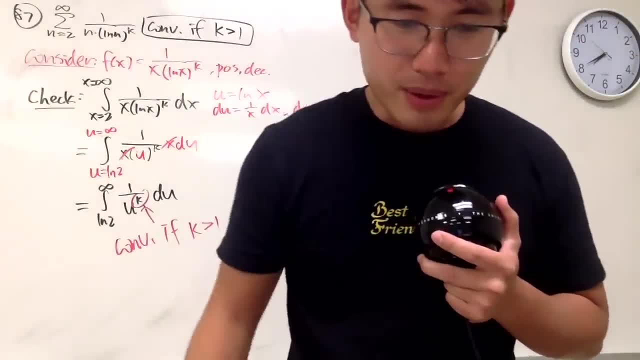 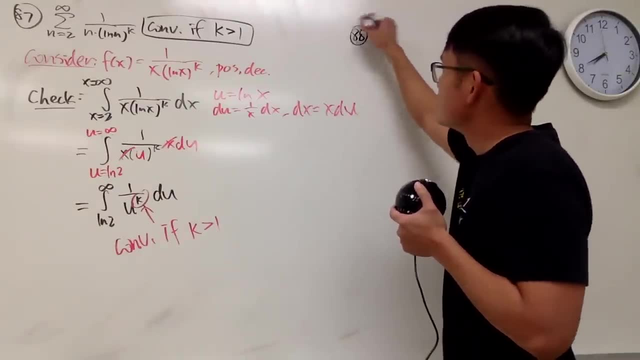 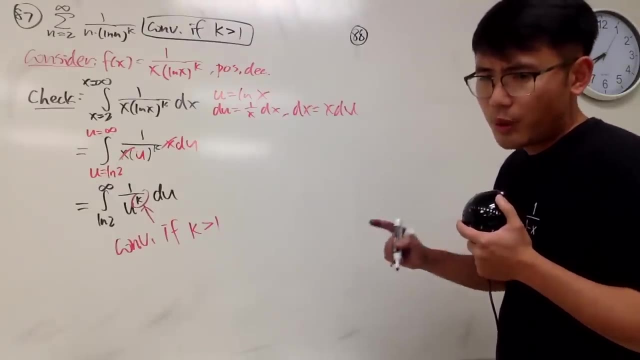 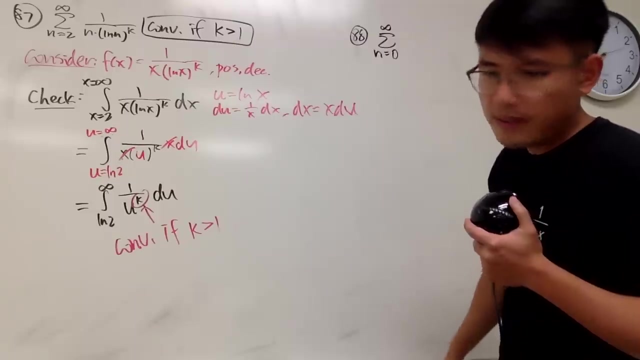 Can Write A Lot Of The Series Questions. All That. I Just Realized I Haven't Drink Anything For The Past, Some As And Goes From. 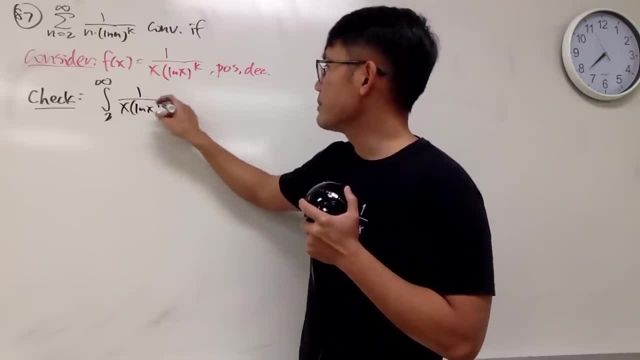 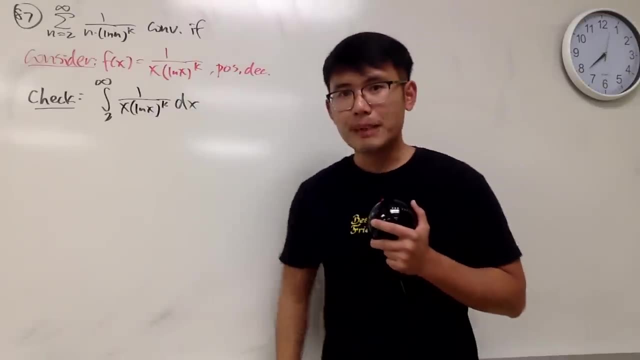 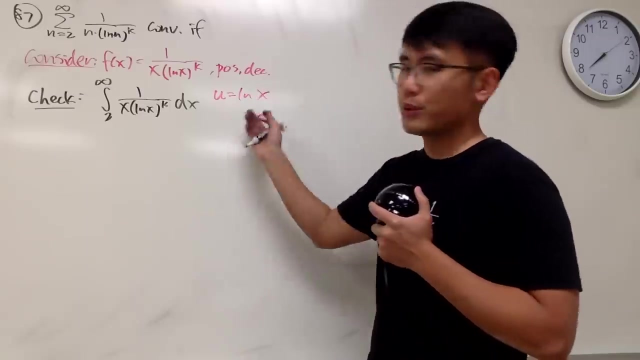 1 over x parentheses. ln x to the kth power dx. To do this, we will do integral, no U substitution, it will be enough, right? So do u sub, let u equal to ln x, and then you do the rest, and we'll do this in your head. 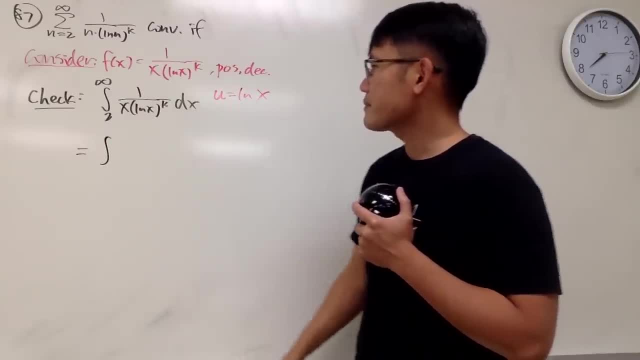 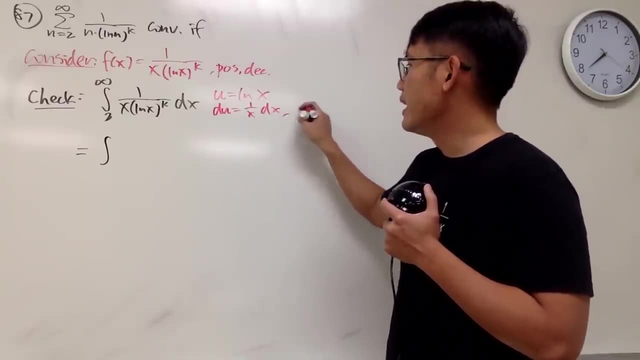 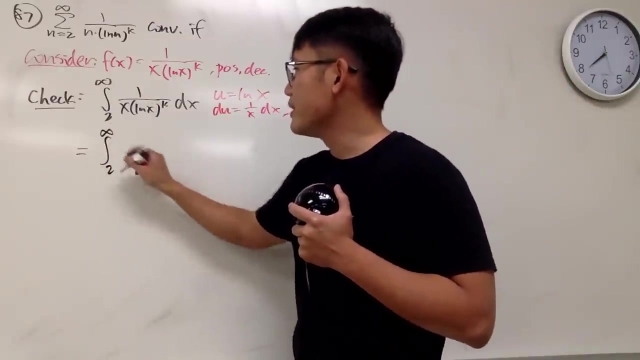 This right here is equal to the integral of. okay, I'll just do it for you guys. du is equal to 1 over x dx and dx is the same as x du. Okay, you see that this right here is 2 to infinity and you get 1 over. 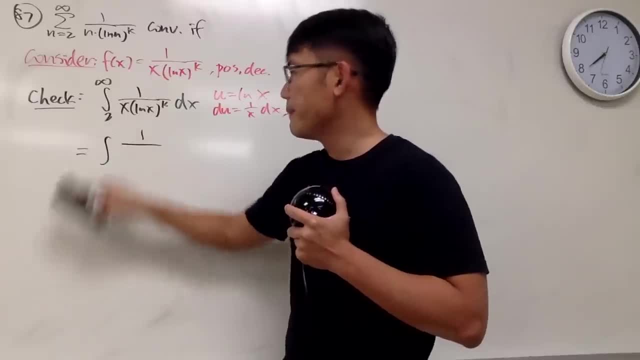 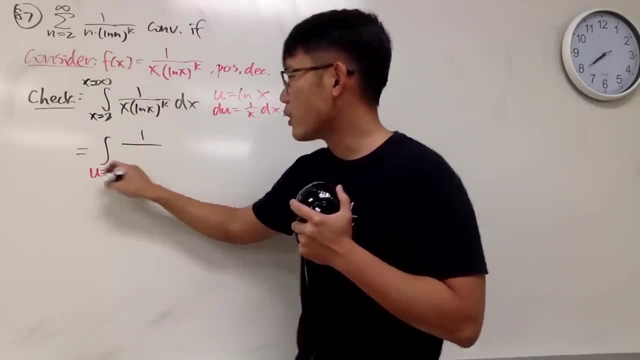 sorry, not 2 to ln. infinity x goes from 2 to infinity, but let's take care of this. in the? u world u will go when you plug in 2, into here you get u is ln 2.. 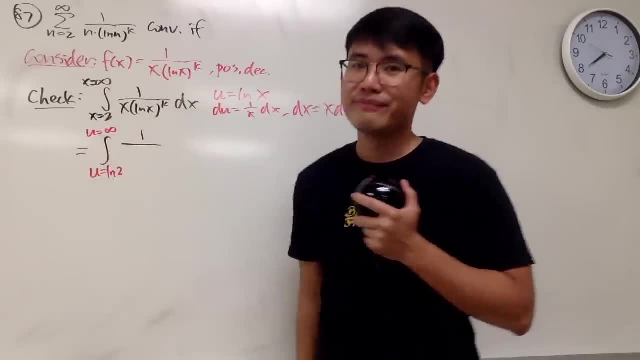 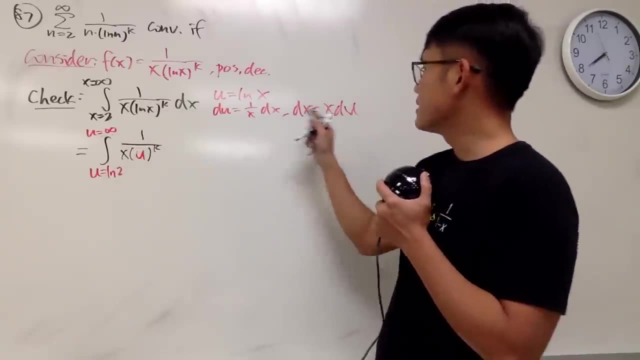 Plug in infinity, here u will be infinity. And then here we have the x parentheses: u k is still k and this guy is x du, so let me just put down x du. So cancel This out, Alright. 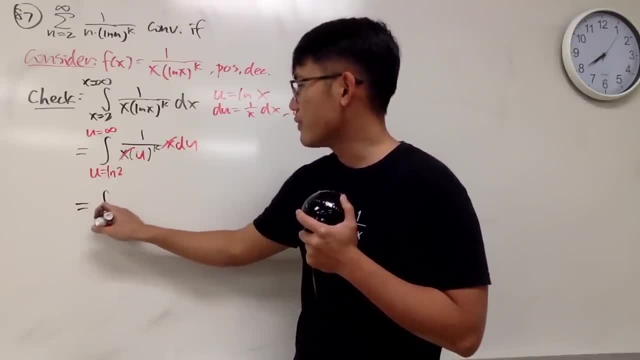 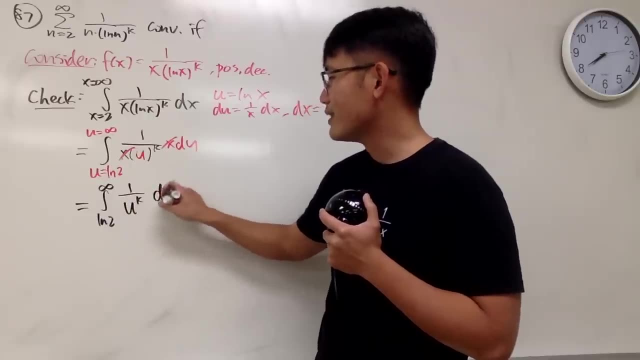 So in this case you will see that we actually just get the integral from ln 2 to infinity in the? u world and we have actually 1 over u to the k's power du. Yes, we have talked about this before. 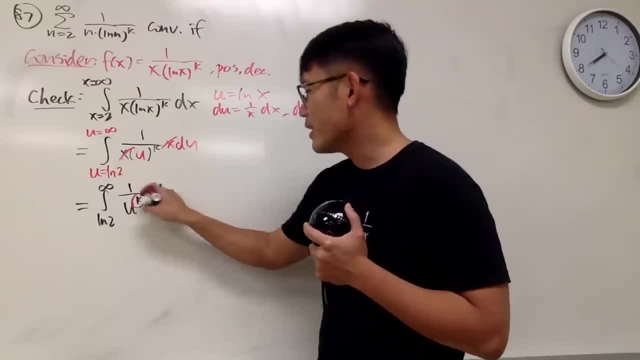 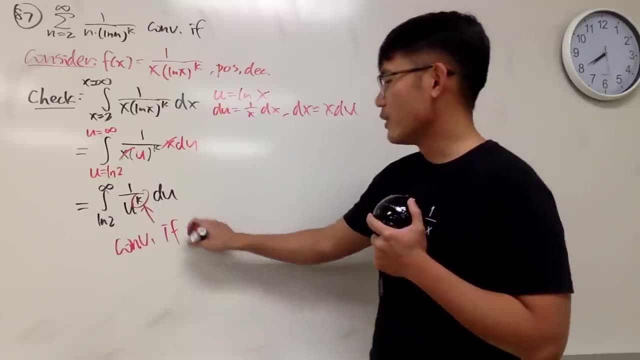 This is the p integral, the p test for the integral right, This right here we know: converge if the exponent here is greater than 1.. So converge if k is greater than 1.. 9, equal to right. So same thing here. 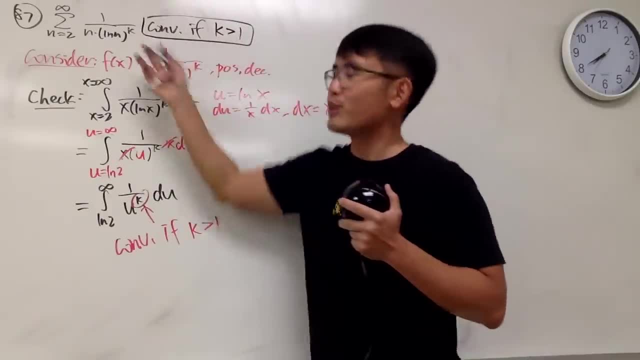 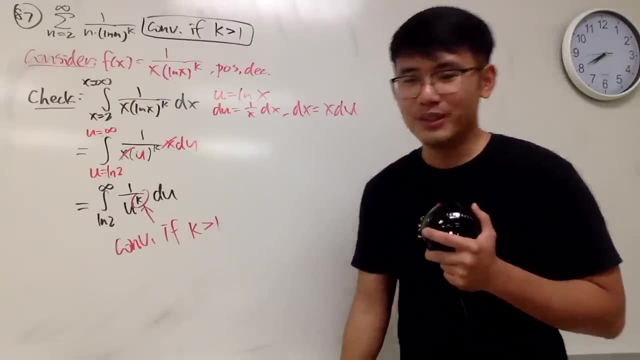 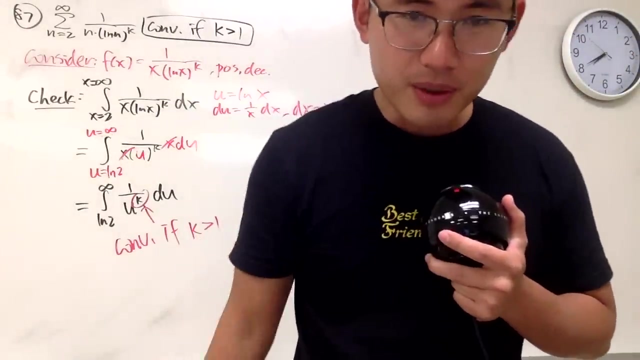 If k is greater than 1.. Huh, so cool, isn't it? So if you know something like these things, you can write a lot of the series questions, all that I just realized. I haven't drank anything for the past 5 hours and I just keep talking, talking. 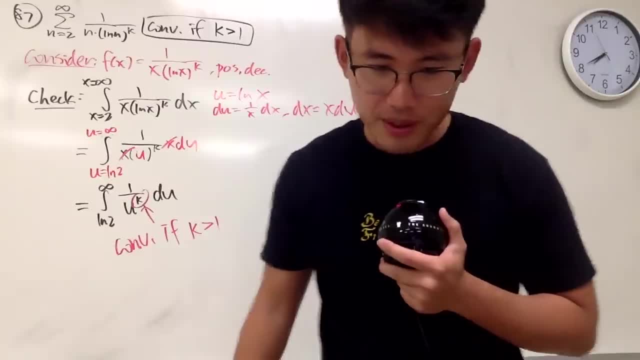 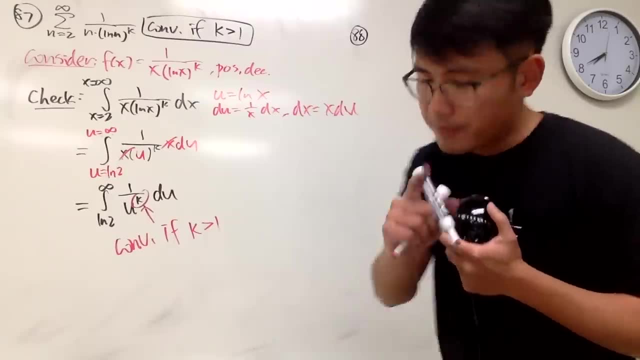 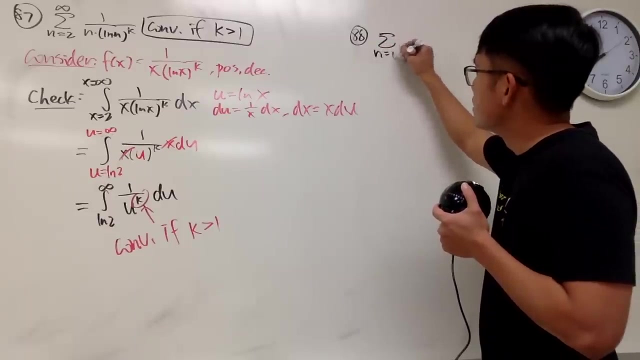 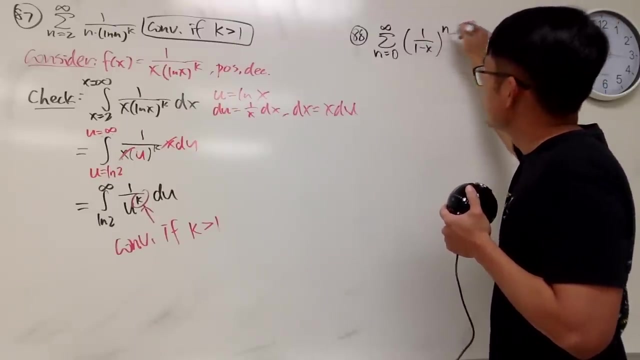 Okay, 5.15,. I'm not going to say too much, I'm going to just finish it. I want to see if I can finish this in 6 hours. I don't think so. Okay, for what value of x will the series, the sum as n goes from 0 to infinity, of 1 over 1 minus x to the nth power, converge? if what? 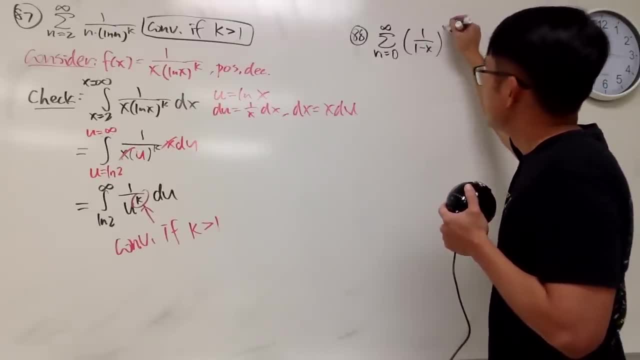 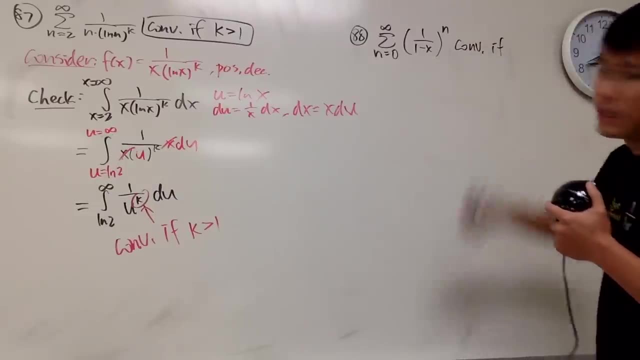 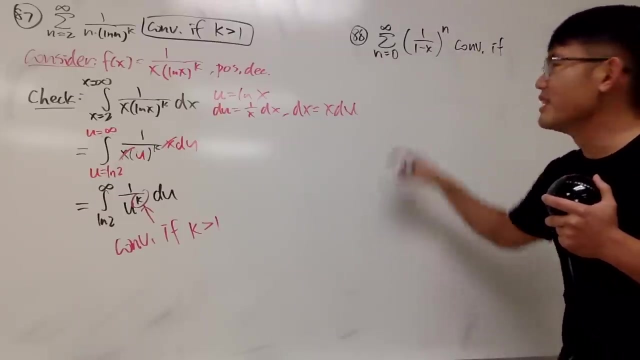 Zero To Infinity Of One Over One Minus X To End Power Converge. If What? Now, Right Here, You Can Use The Root Test. 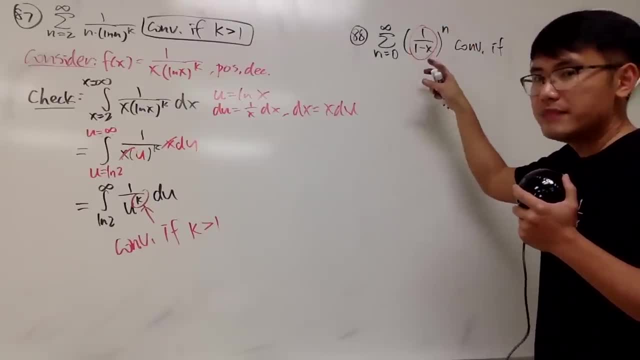 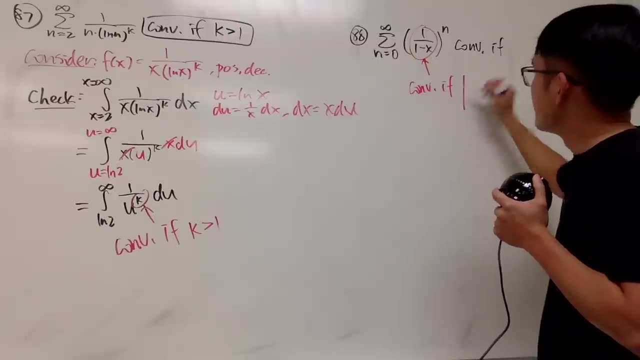 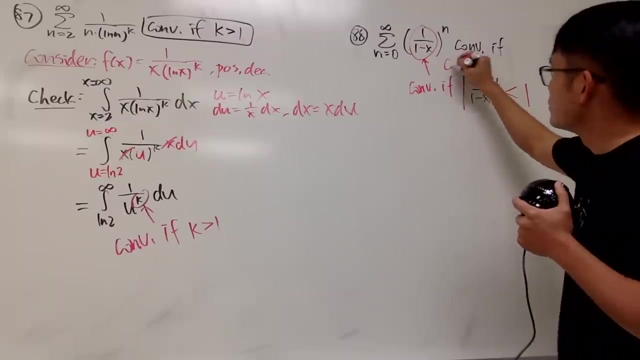 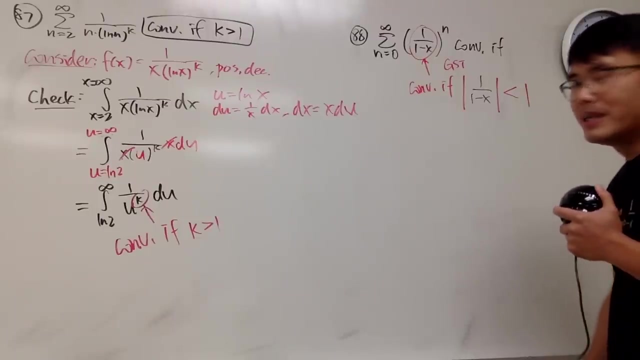 But For X Is Just A Number, It Has Nothing To Do With N And Take This To The End Power. So We Know This Right. 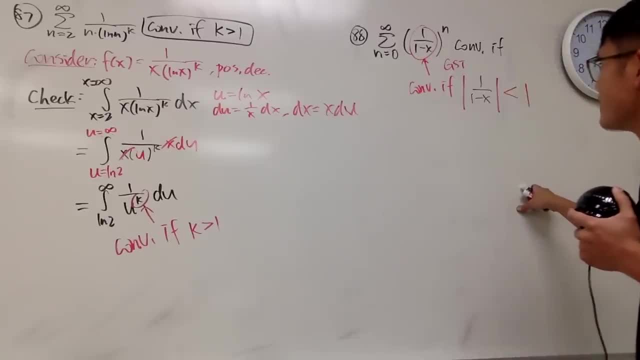 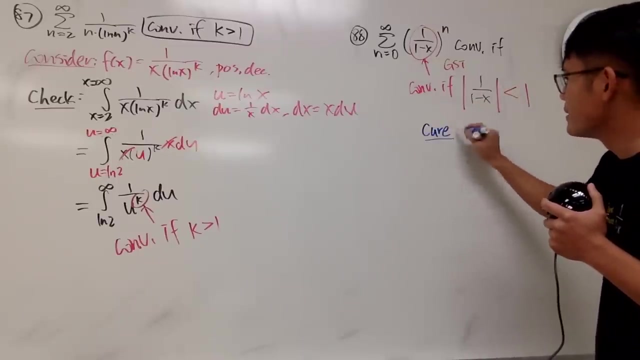 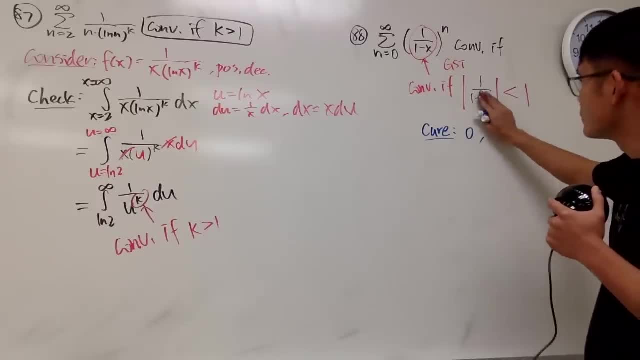 Is One, X Is One, So We Know. Next, You Also Care About Two, Because If X Is Two, Then One Over One Minus Two. 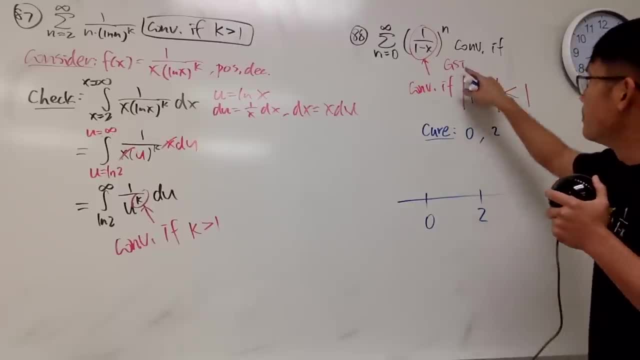 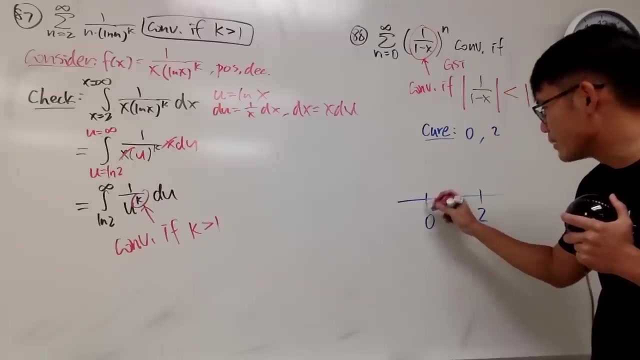 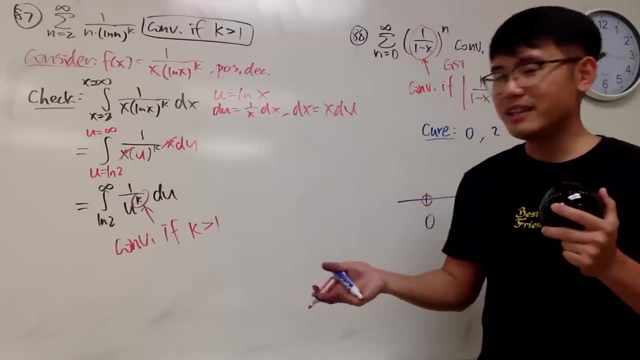 Is Negative One. Absolute Value Of Negative One Is One, So This One Is Not Good. We Care About These Two Numbers, But We Don't. 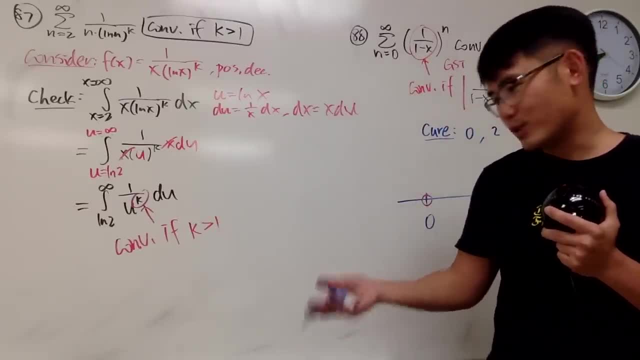 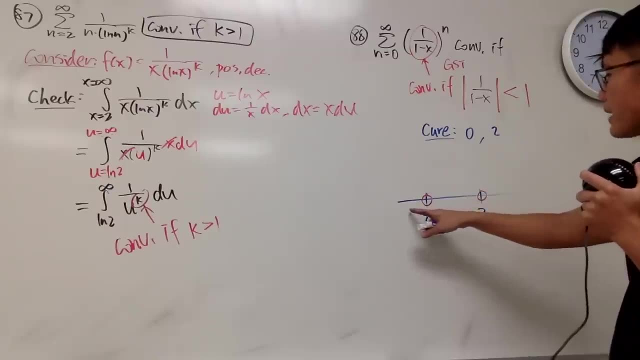 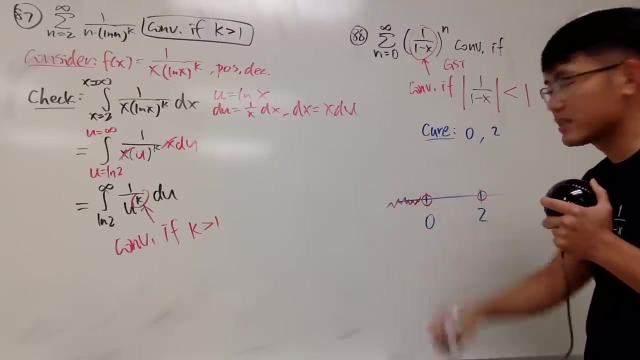 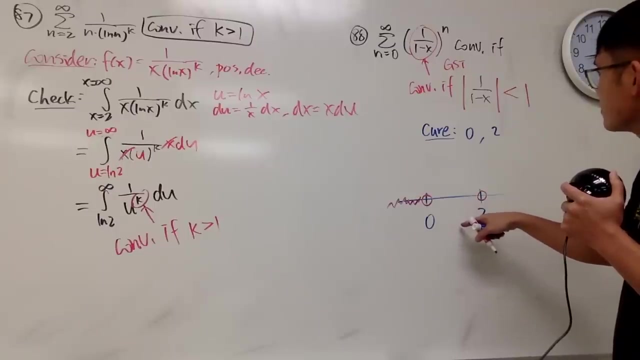 Want To Have Them. So Let's Put On The Open Circle Here And Open Circle Here. It Works, So This Work, It Checks Right. So 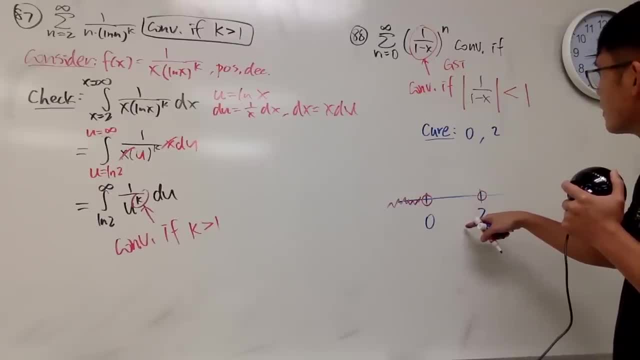 Just Check Negative One: Any Number Works. Plugging, Let's Say One, Doesn't Make Sense. Okay, Plugging, Let's Say One Half. So The Truth. 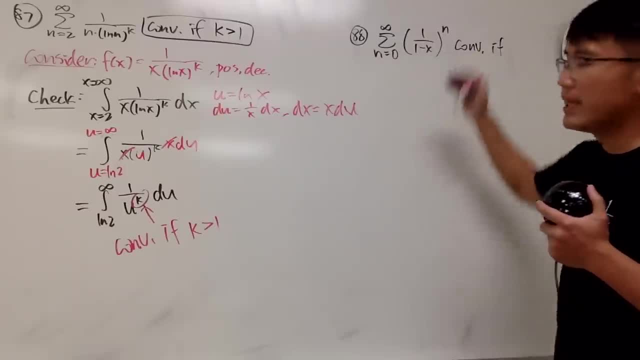 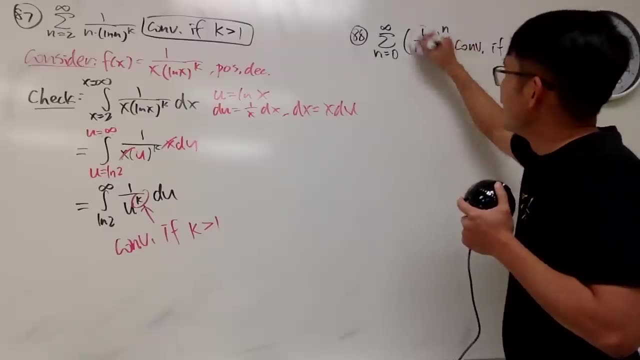 Now, right here you can use the root test, but the idea is that this is also the geometry test, so you don't know what the inside is. So up to you, I will use the geometry test right, Because again you have some number. x is just a number, it has nothing to do with n. 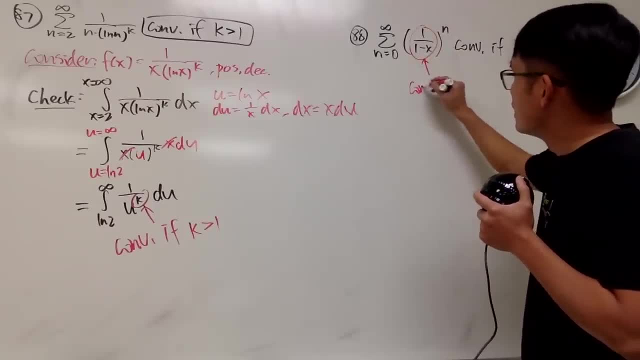 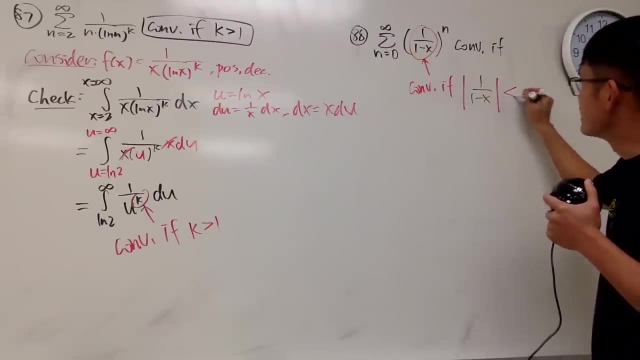 and take this to the nth power, so we know this right here: converge if the absolute value of 1 over 1 minus x is less than 1, geometric, like GST, based on the geometry series test, And now this is not that bad at all to work with. 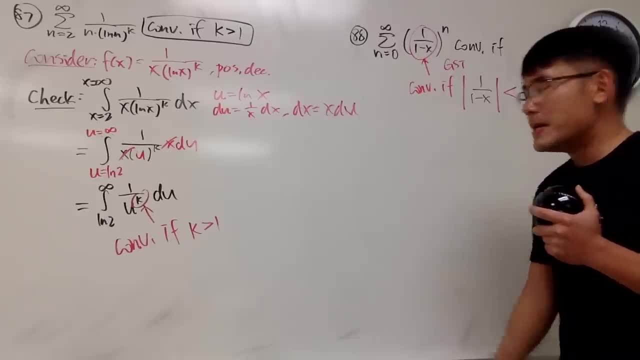 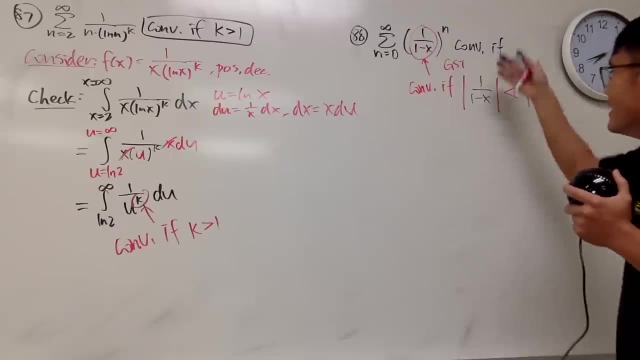 And actually I will show you guys how I can do this right. Hmm, You guys depends on how you want to do it. If you want to do the nonlinear absolute value inequality, it takes some time. so this is how you can do it. 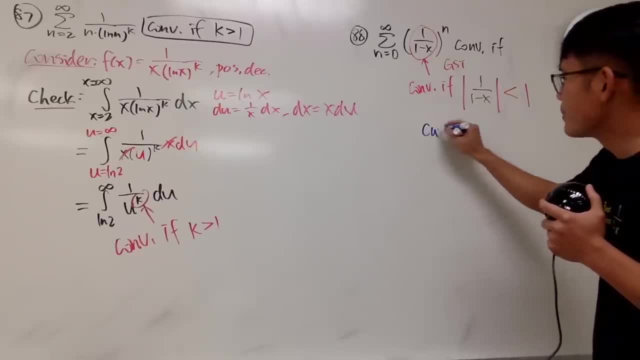 How can you make this equal to 1?? I will just tell you guys two numbers that we care, right, We care about. x is equal to just care about. how can you make this equal to 1?? Well, I'm not going to say 0, just say 0. 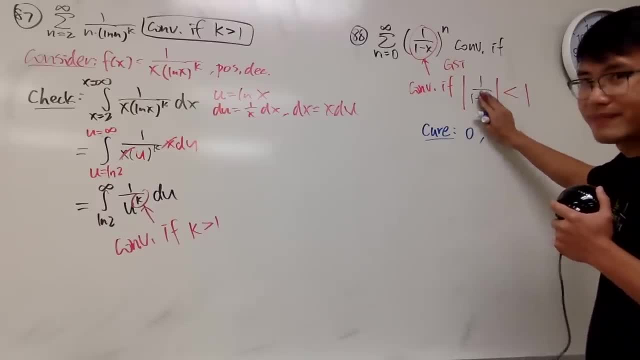 I mean x equal, I will say 0.. Because I don't want to say 0. Because if x is 0, this is 1. So that's like on the borderline. so you care about that. Next, you also care about 2.. 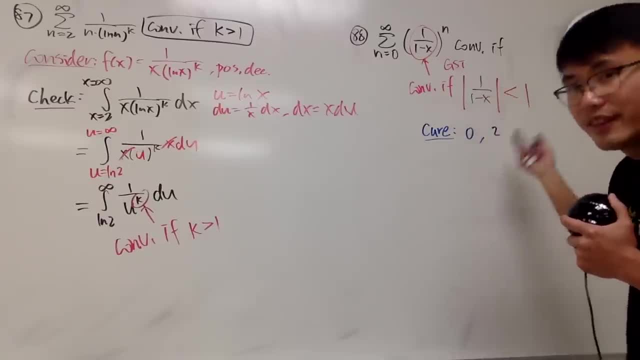 Because if x is 2, then 1 over 1 minus 2 is negative 1.. Absolute value of negative 1 is 1.. So this is still on the boundary right. So you care about these two numbers And what you are going to do next is just draw the number line, put down 0 and 2.. 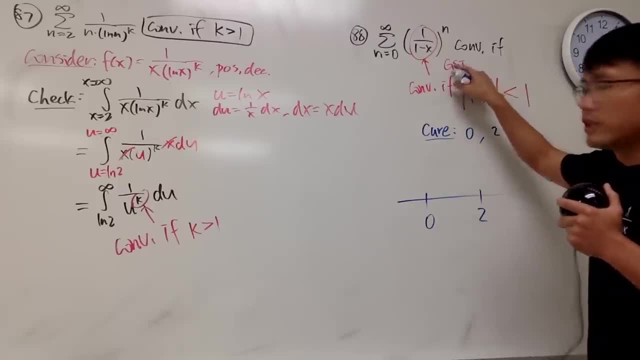 Well, as we all know, based on the best friend, the geometry series test, we do not include the endpoints of the interval. So if this is exactly 1 or negative 1, it's not good. We care about these two numbers, but we don't want to have them. 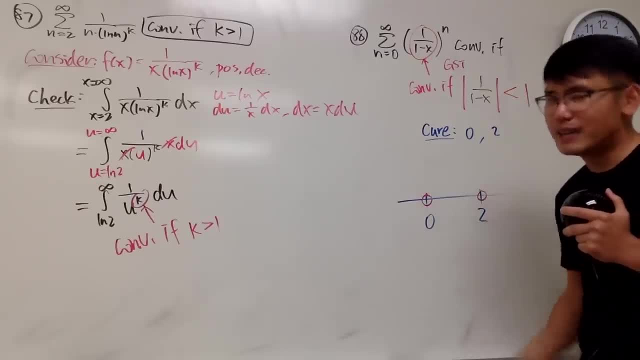 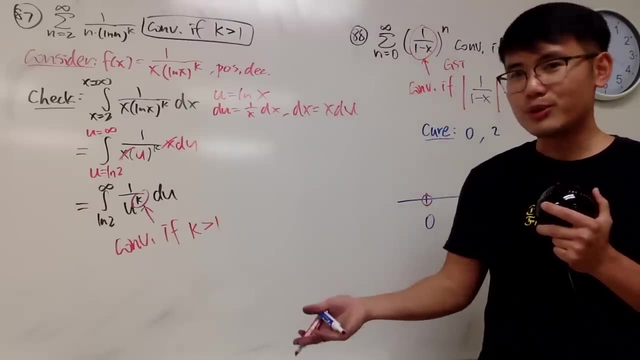 So let's put down the open circle here and open circle here. I know it's weird. This is like saying when somebody turns into 18, the parents will say: you know, Johnny, I care about you, but I don't want to have you in the house. 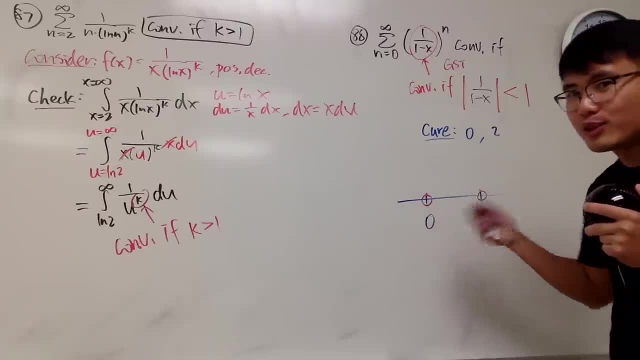 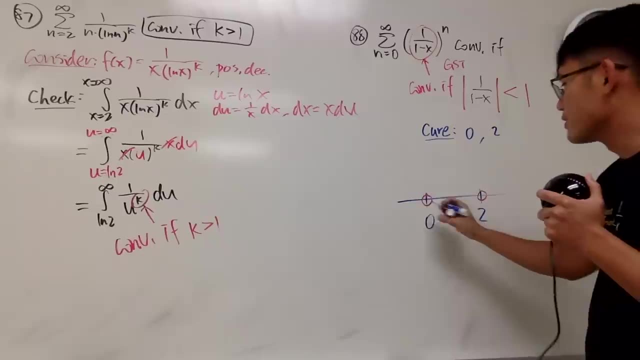 That's pretty much the same idea, okay. Anyway, now you're just going to plug in number and check. For example, plug in negative 1 here, 1 over 1 minus negative 1, which is 1 half. So that means it works. 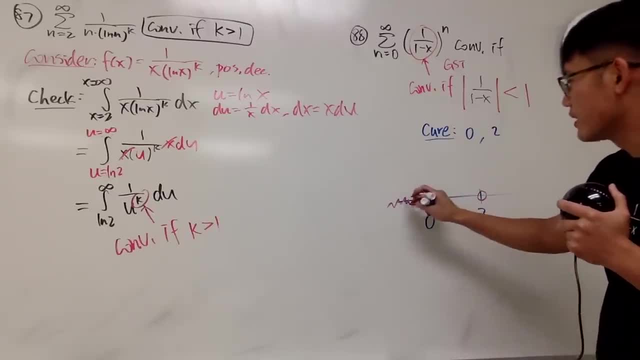 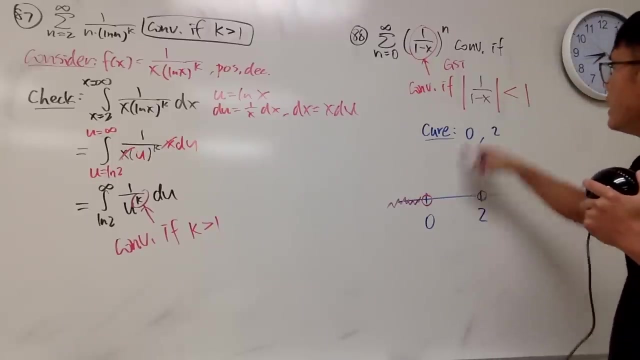 So this one here checks right, So you just check negative 1.. Any number works. Plug in, let's say 1. doesn't make sense, Okay. Plug in, let's say 1 half, And you get 1 over 1 minus 1 half. 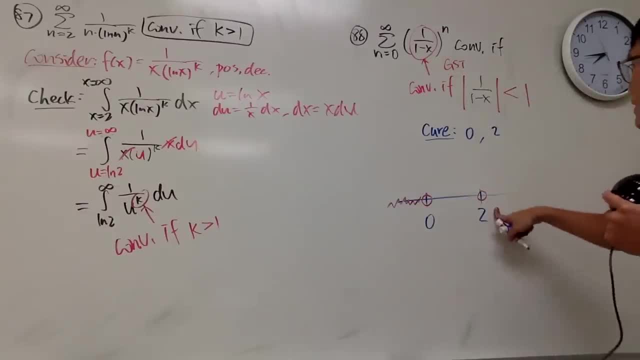 Actually it's 2.. So this interval is no good. And lastly, let's say: plug in 3.. 1 over 1.. 1 over 1 minus 3.. Absolutely for you, that is actually good. So we have all this. 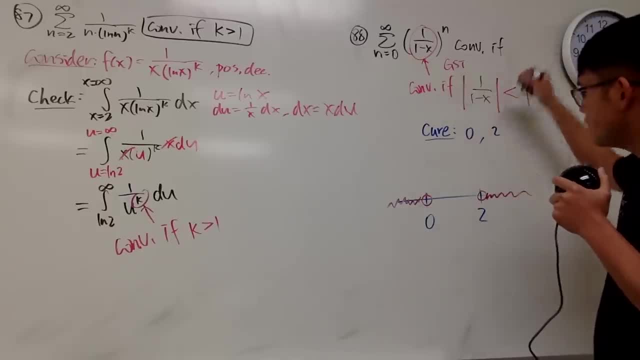 So the truth is this, right here converges if x. Okay, Now this is the bizarre part. Oh yeah, 0, 0 doesn't work. Yeah, 0, 0 doesn't work, So yeah, So this converges if x is less than 0 or greater than 2.. 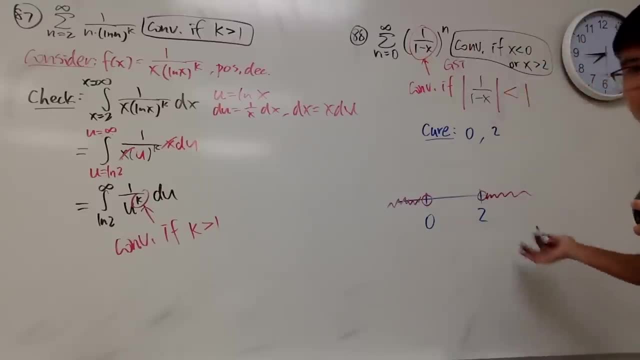 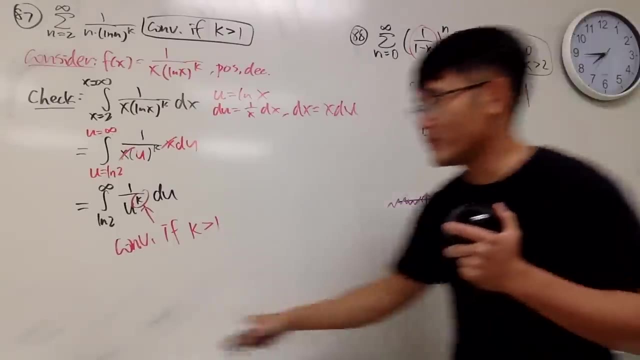 Woo-hoo, Done Right. So just do these kind of things, And I think it should be pretty okay to just draw this kind of algebra or like work for the inequalities. Okay, Number 89.. Very, very similar Number 89, right here? 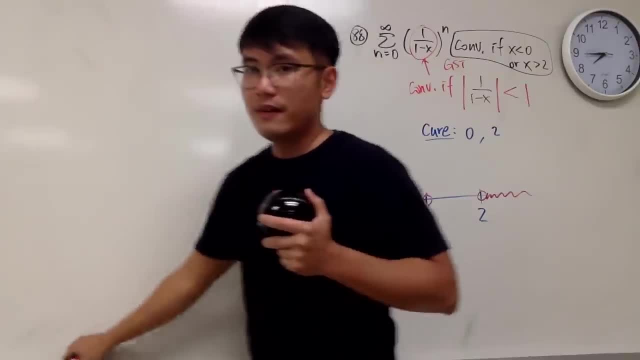 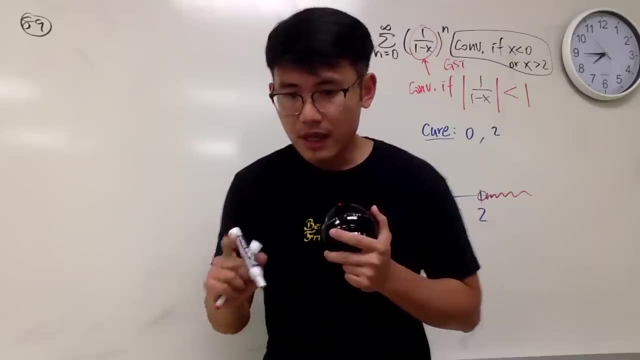 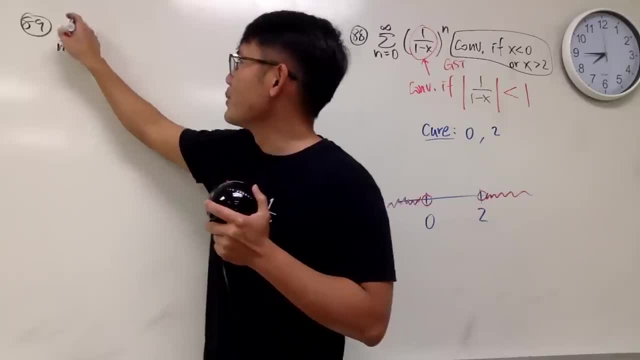 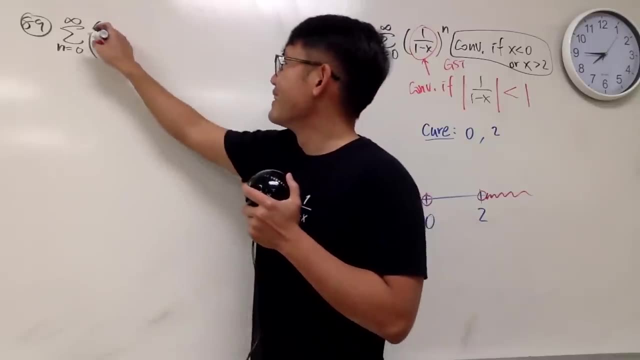 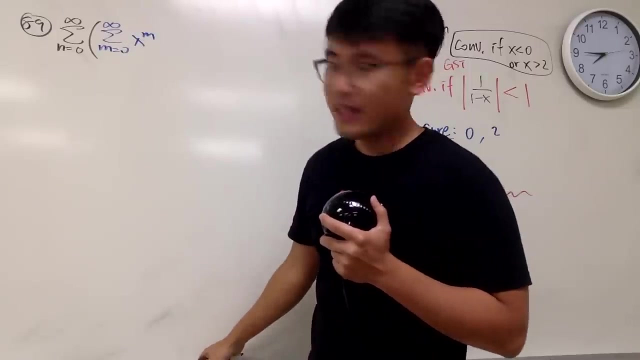 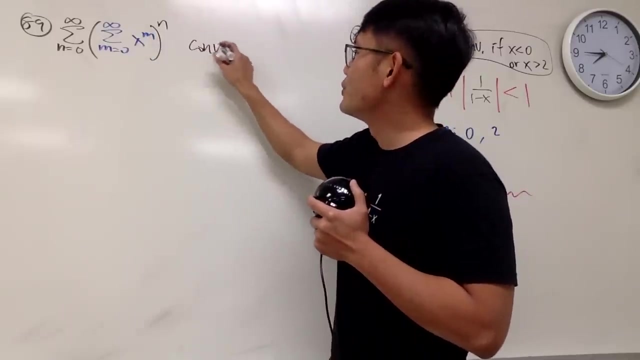 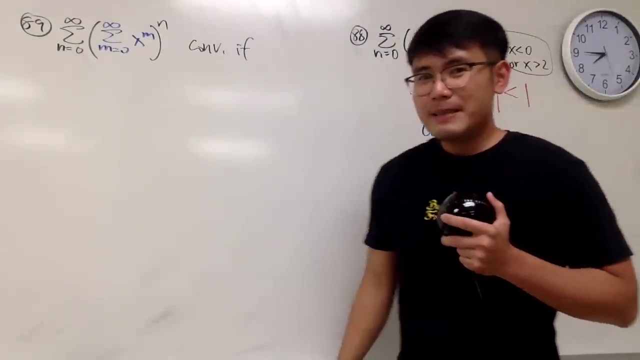 Number 89.. Maybe the sum of m goes to infinity x, to infinity x to the m. then I would take this radius to the and power this right here will converge if what? And, by the way, I comfortable to this question on my own, just an extension of that. Be careful with this one. Now here we go. First of all, we 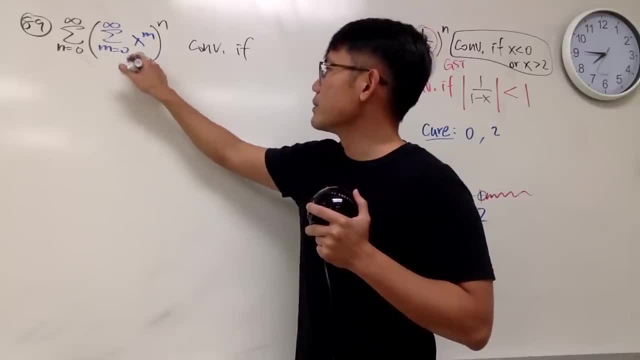 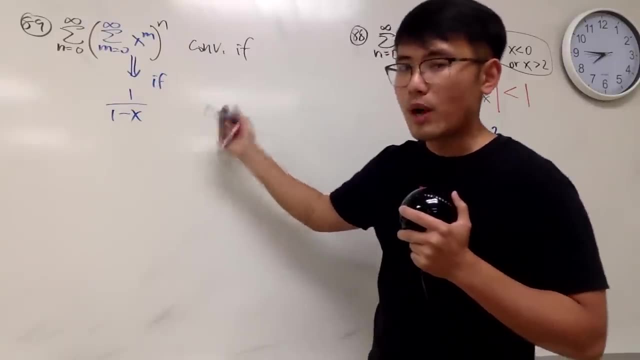 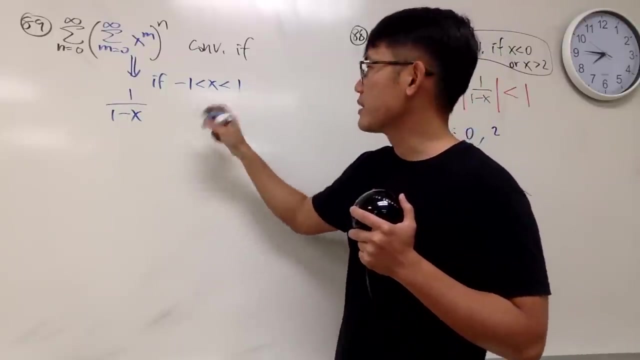 know this right here- converges to- let me just do like this- converges to 1 over 1 minus x if absolute value of x is less than 1.. So we can put down negative 1, this: well, x is between negative 1 and 1.. So this is a condition that we need right. We need this. 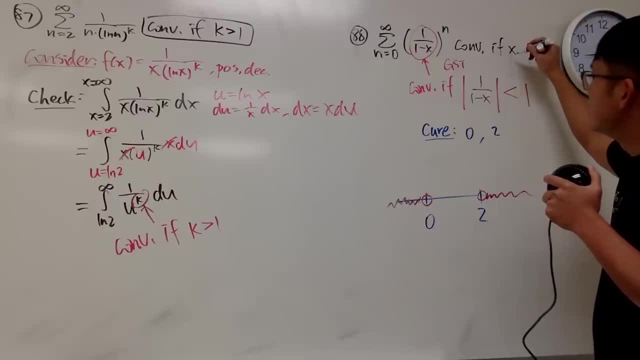 Is This Right Here? Converges If X, Okay. Now This Is A Bizarre Part. Oh Yeah, Zero Zero Doesn't Work. Zero Zero Doesn't. 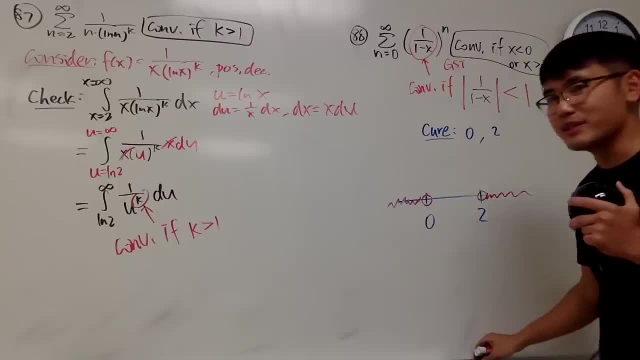 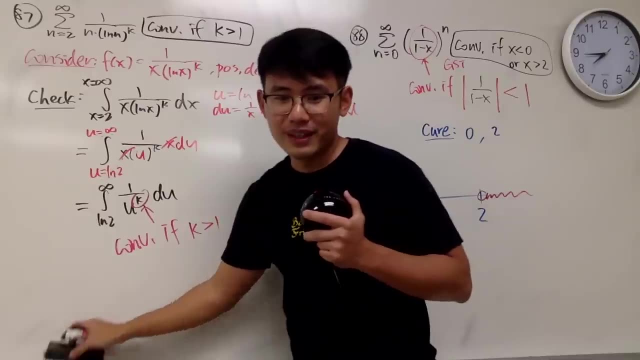 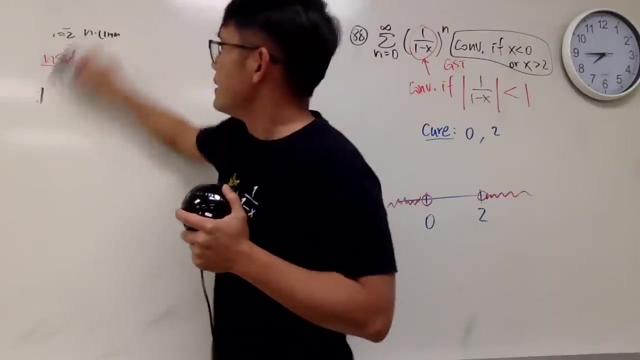 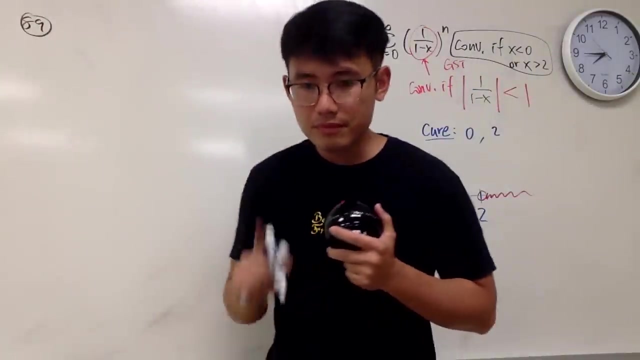 Work So Yeah. So I Think It Should Be Pretty Okay To Just Show This Kind Algebra What Like Work For The In Qualities Okay. 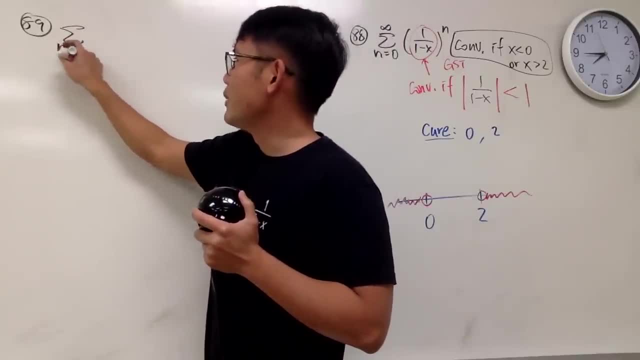 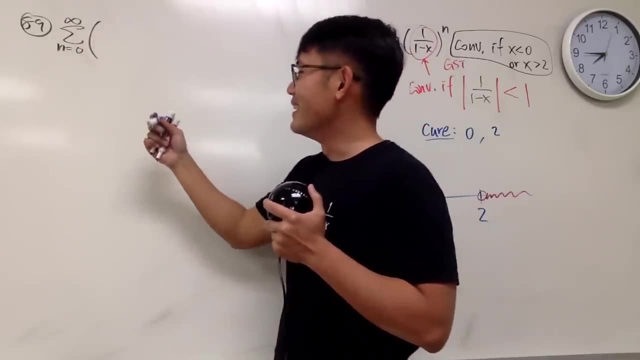 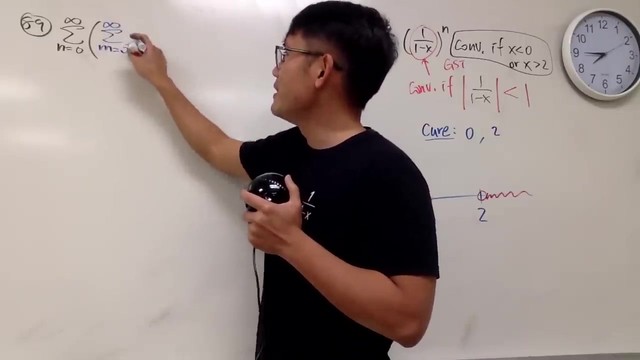 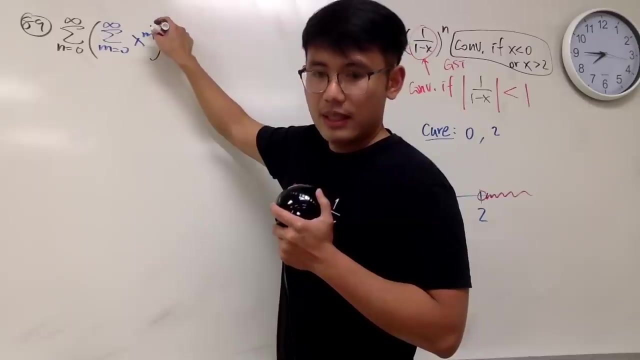 Number 89.. Very, Very Similar Number 89.. Right Here We Have The Best Friend. The Song As M Goes From Zero To Infinity X To. 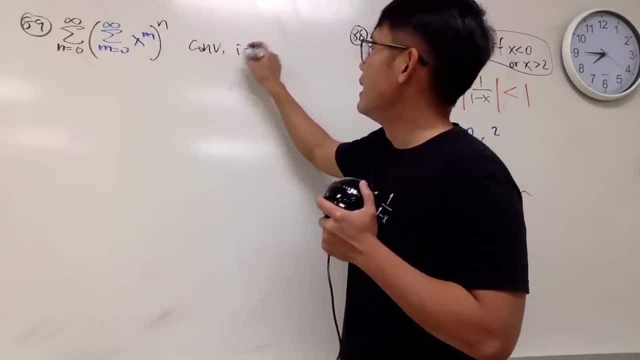 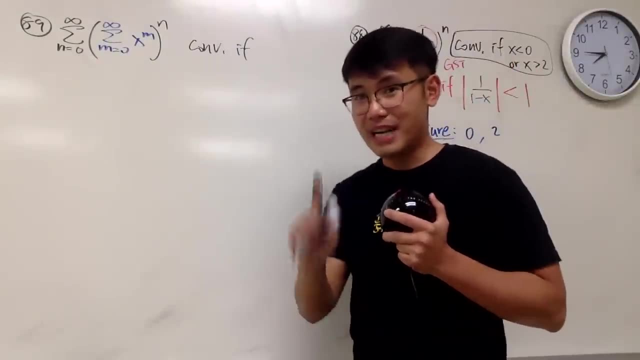 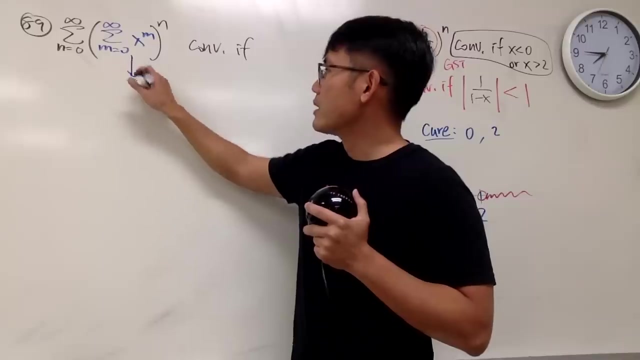 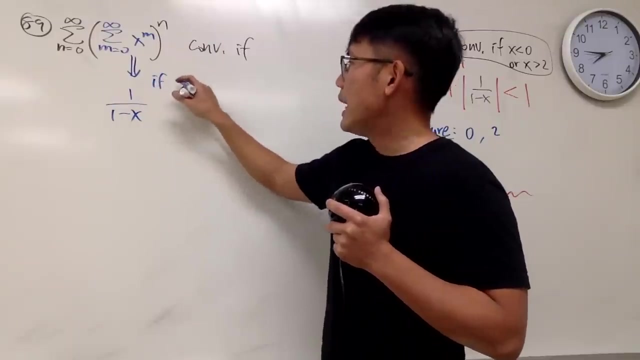 The M, And Then I Will Take This Race To The Power. This Right, First Of All, We Know- This Right Here Converges To Just 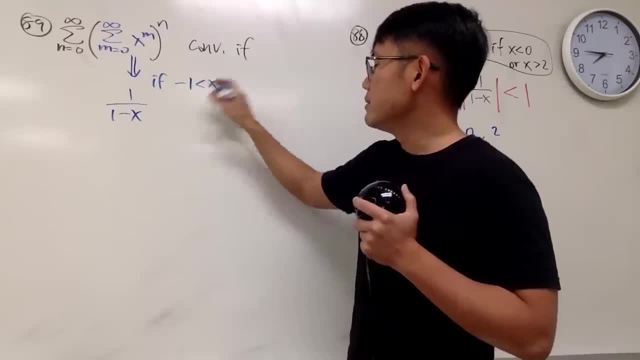 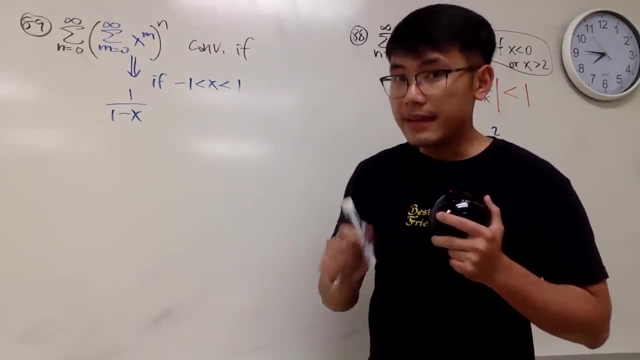 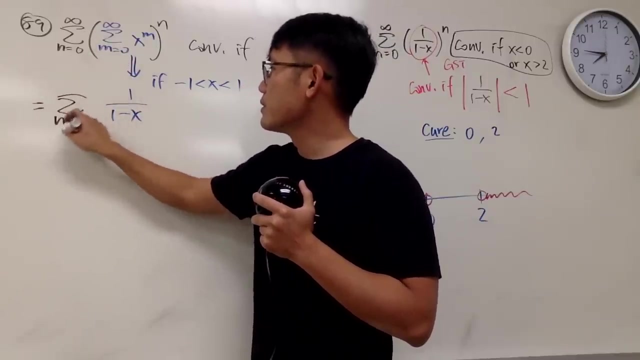 Like This: Converges To One Over One Minus X. If Absolute value Of X Is Less Than One, So Zero To Infinity, And Then To. 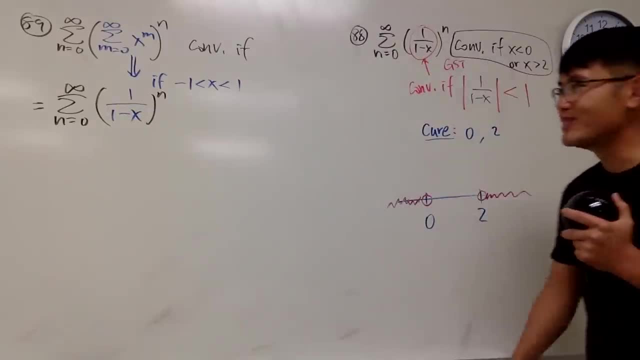 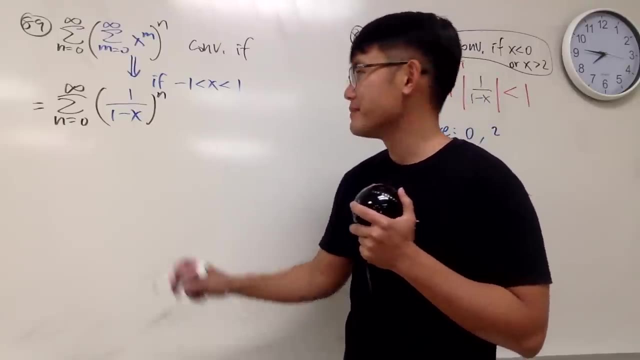 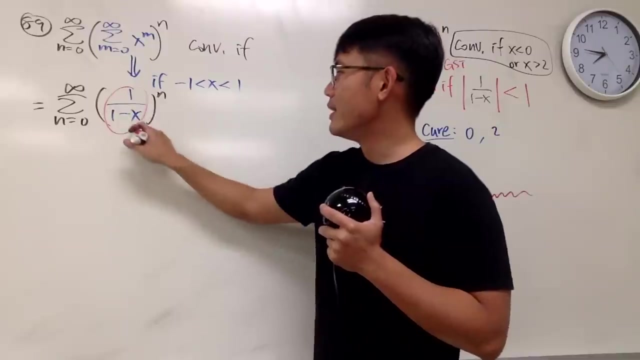 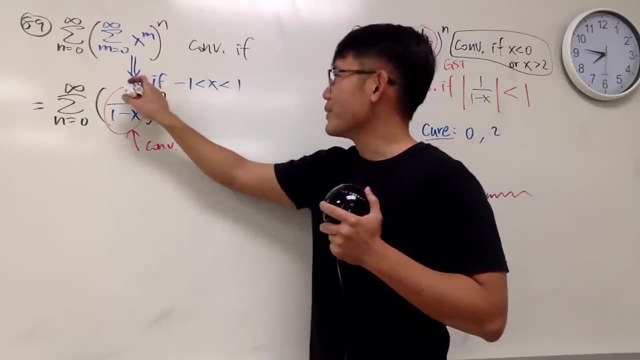 The End Power Like That, So You Can Make This Change Under This Condition. Yes, We Can Do This Kind Of Things Again To You Earlier. 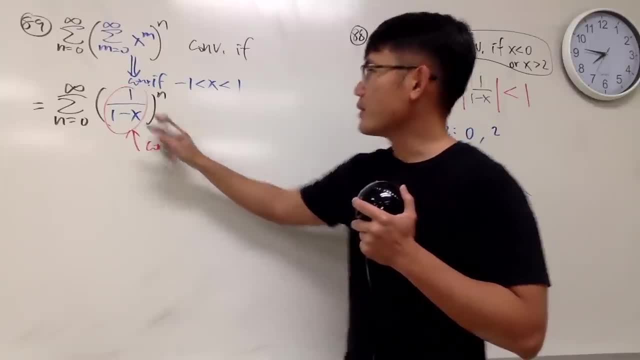 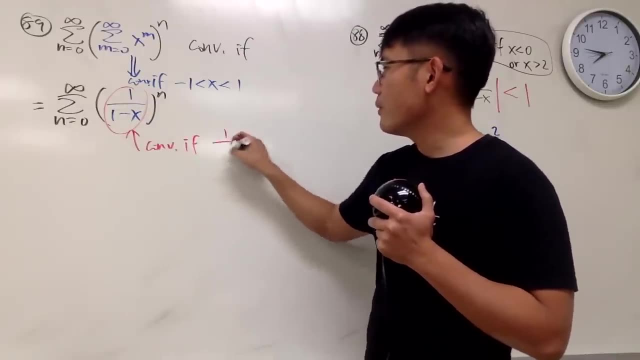 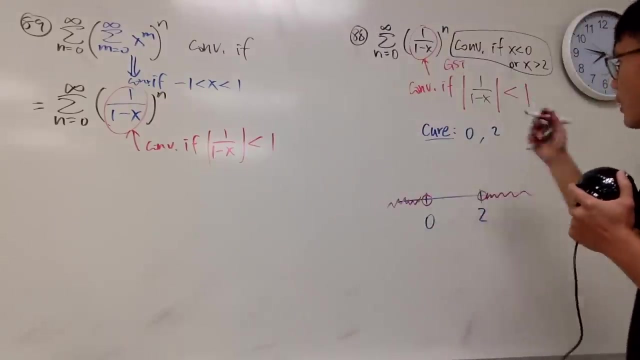 From Here To Here Converge. If So, This Right Here, Come On, This Whole Thing Converge. This Whole Thing Converge, If If One. 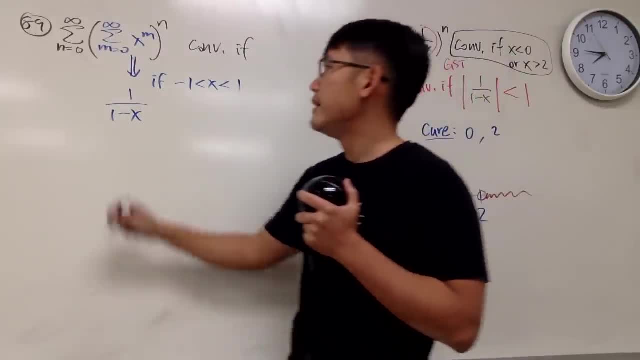 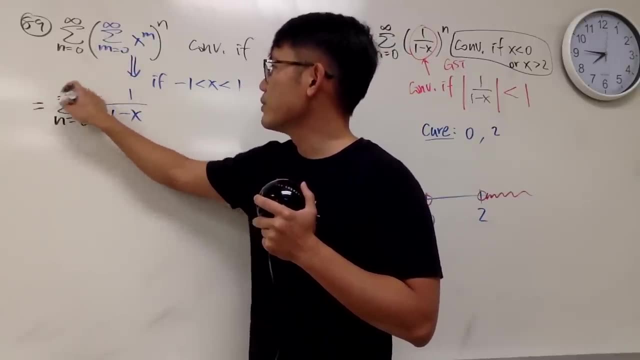 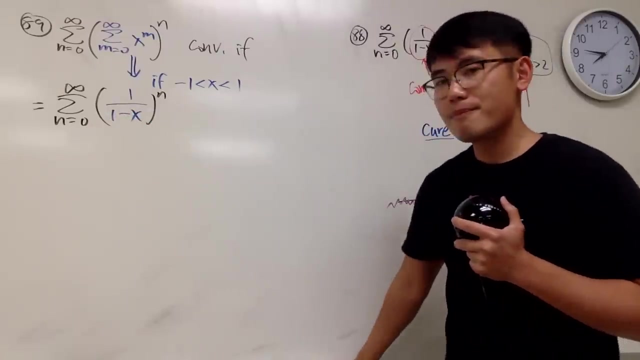 condition, And then you are going to write this down, which is the sum, as n goes from 0 to infinity and then to the nth power, like that, So you can make this change under this condition. Yes, we can do this kind of things again, But be careful this time though. Well, 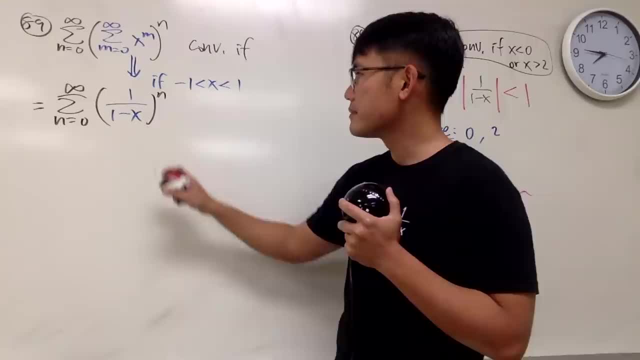 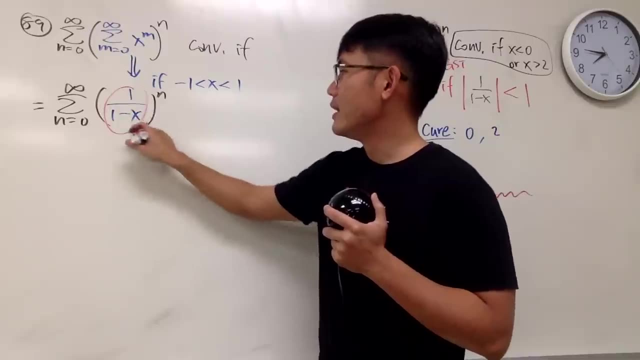 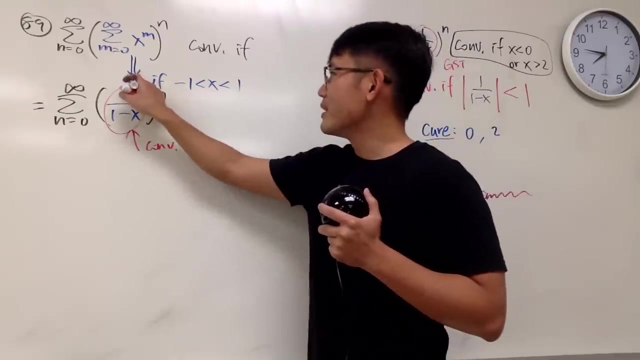 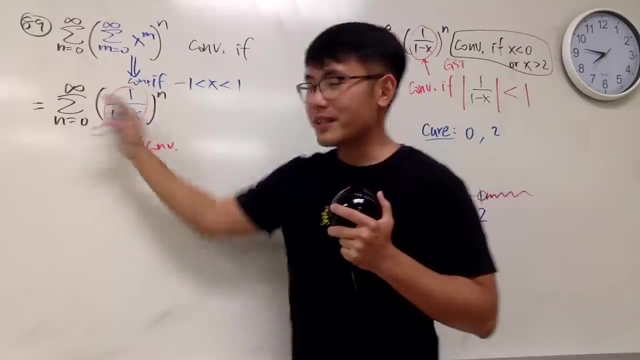 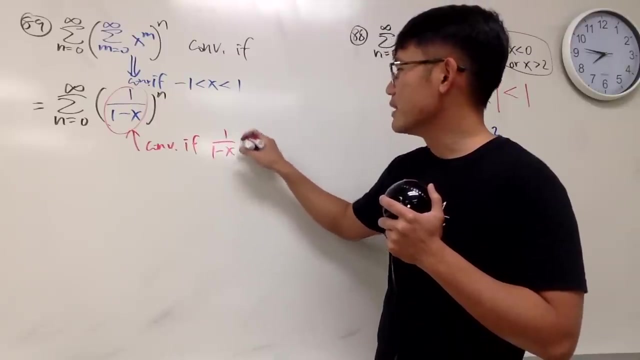 this time we want this Converge. I should also put on converge in blue earlier. From here to here: converge. if so, this right here. well, this whole thing converge, this whole thing converge. If 1 over 1 minus x, absolute value of that is less than 1, right, And based on what we saw. 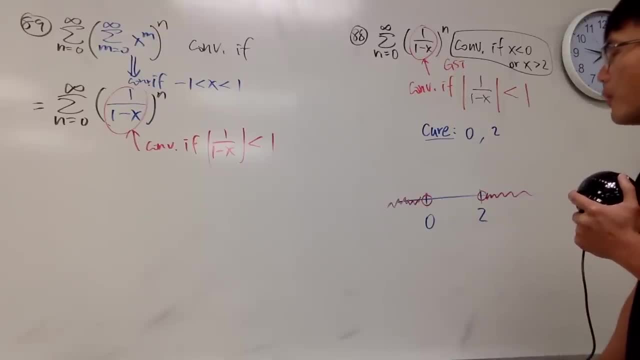 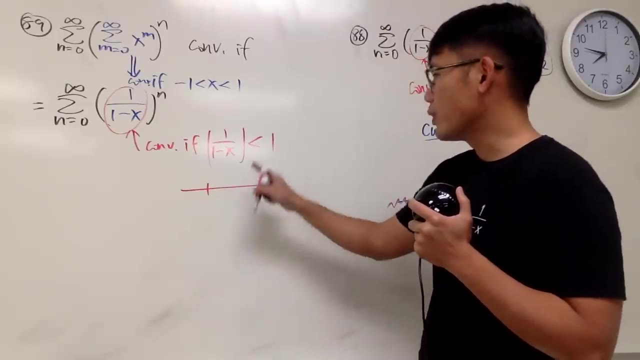 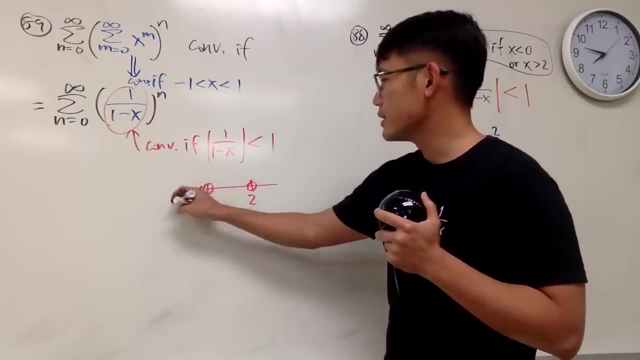 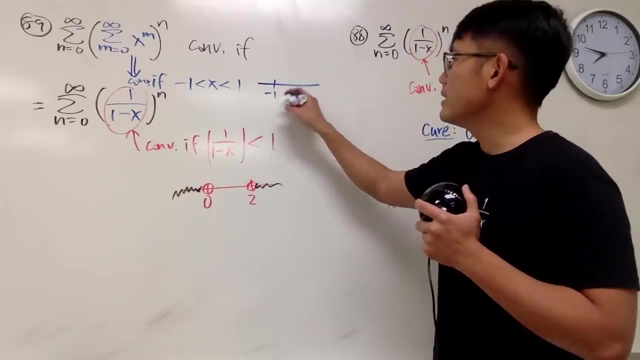 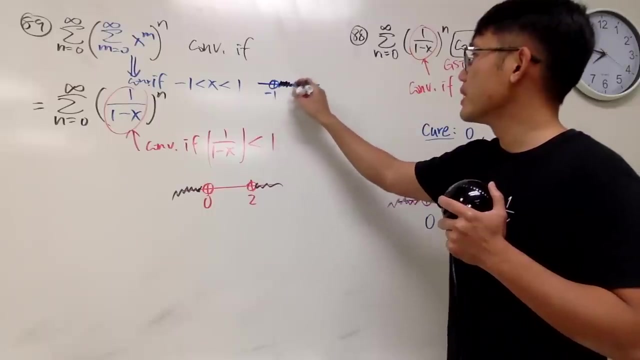 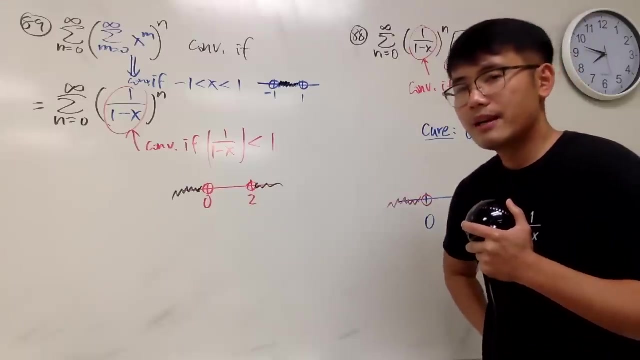 earlier. well, we have this inequality which is for the red one, which is 0 and 2, open, open and you do this, you do that, and earlier. this one right here is technically like this: negative, 1&1 and open, open and in between. okay, so here is the deal here. 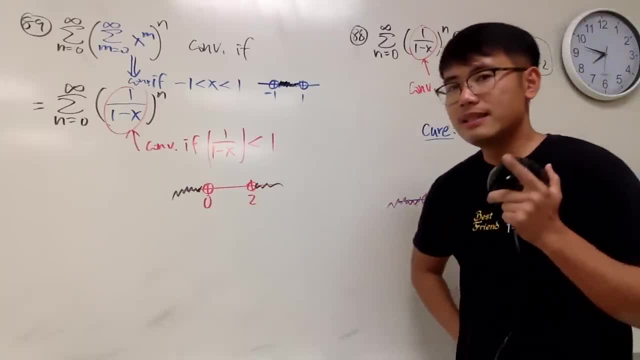 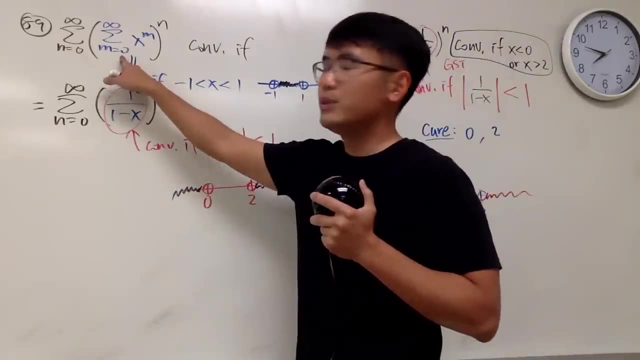 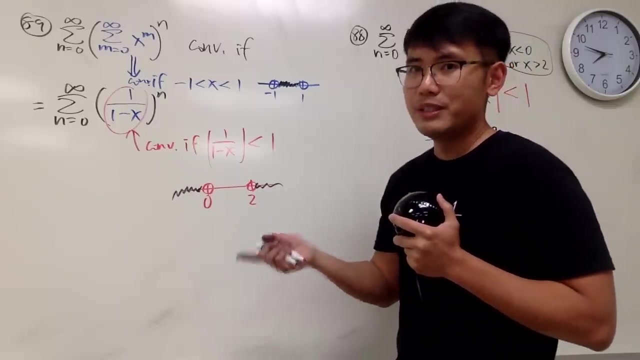 is that deal? it depends on how do you want to do this guy right here, since I put down and is equal to 3 row because, again, this is the best-friend version. right 0 to the 0 in power series is 1.. 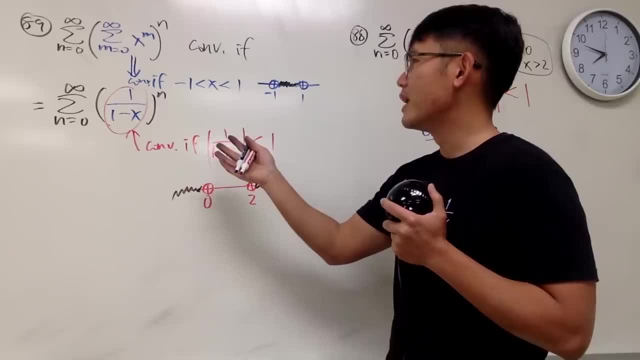 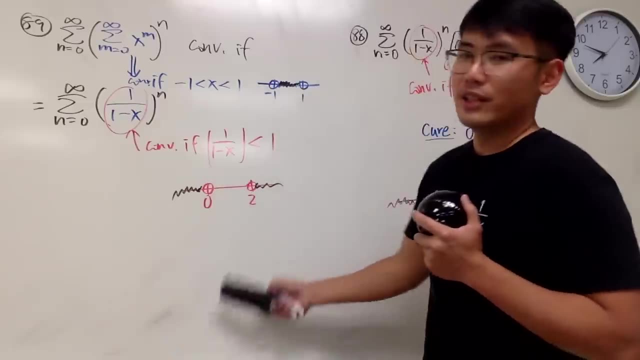 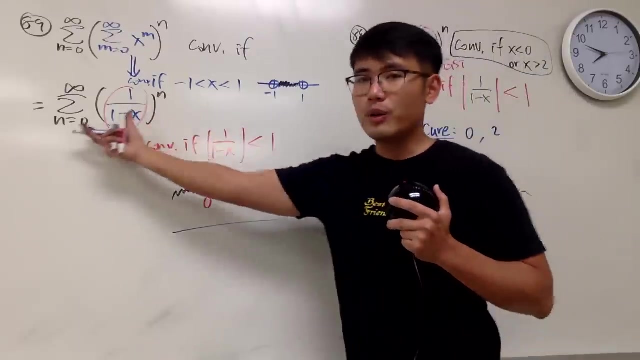 So we can not include that, of course. Yeah, of course we can not include that, never mind, Anyway, just ignore what I said. Alright, so we have these two conditions, So perhaps I will just put this down in this right here. So this is the one from here which is the. 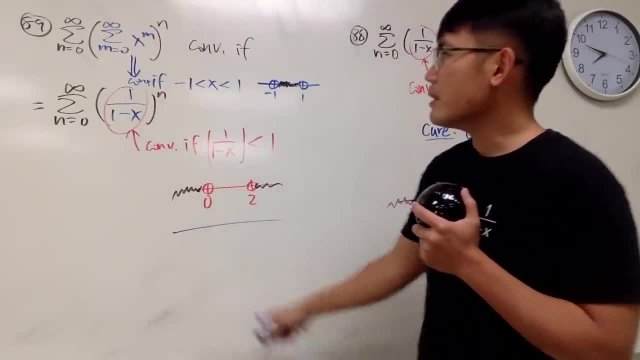 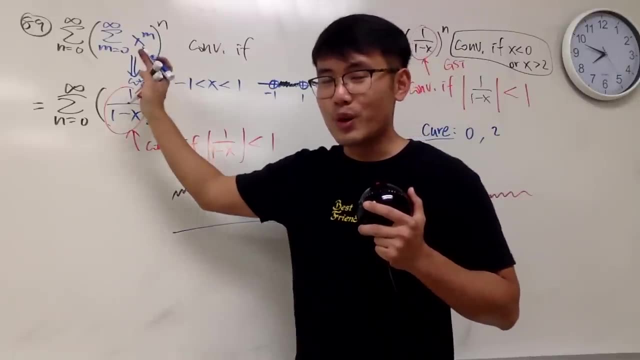 earlier question and this one is from the best-friend: right, If x is equal to 0, technically this, you get 1, right. So you are not going to include 0, 0 is actually not going to work. 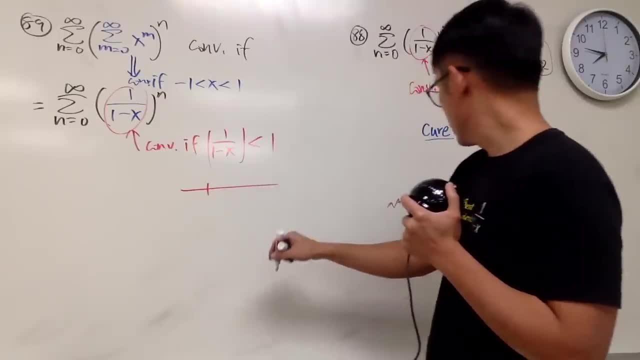 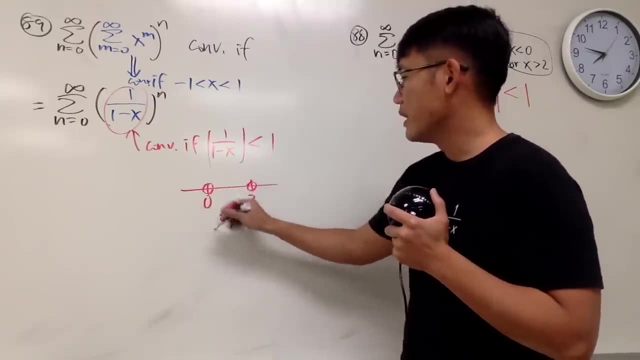 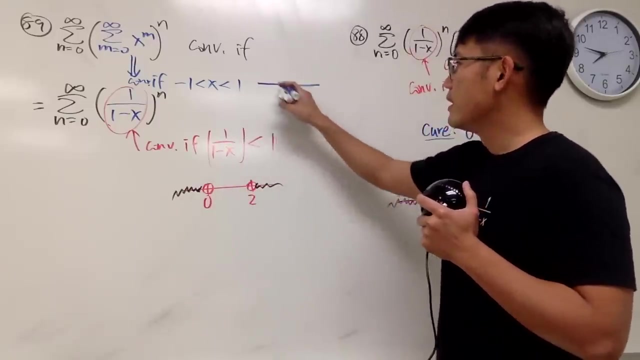 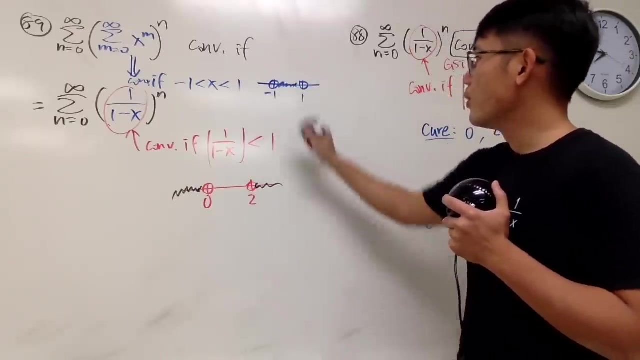 Over One Minus One For The Real One, Which Is Zero, And Two Open, Open, And You Do This, You Do That And Earlier This, 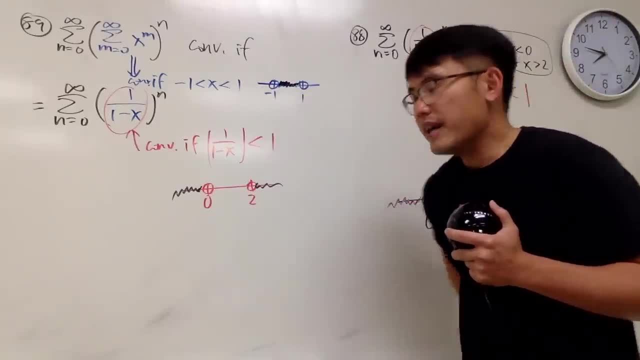 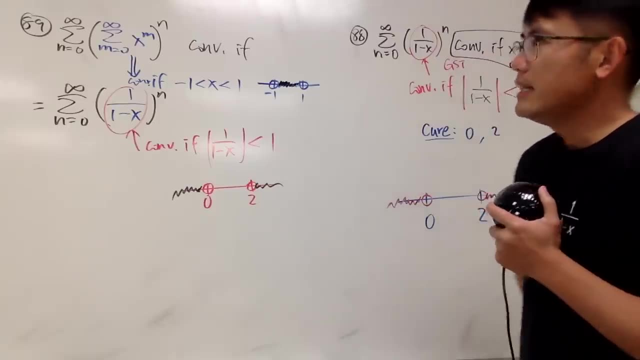 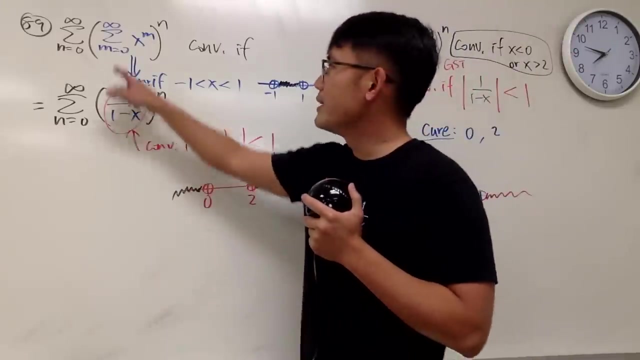 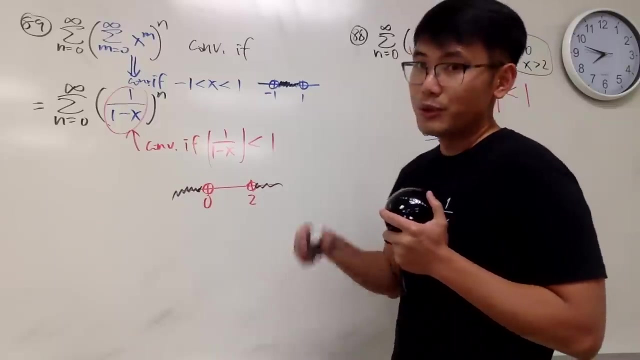 One Right Here Is Technically Like This: Here Is The Deal. It Depends On How You Want To Do This Guy Right Here, Since I 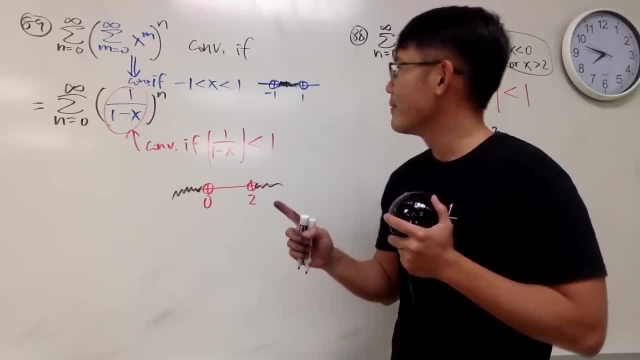 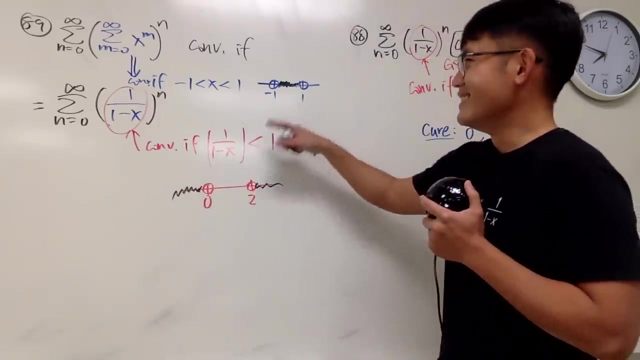 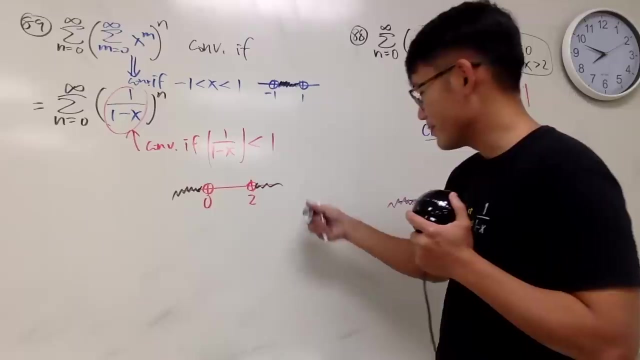 Put Down M Is Equal To Zero, Because, Again, This Is The Of Course, Yeah, Of Course, We Can, Anyway. All Right, So We Have This. 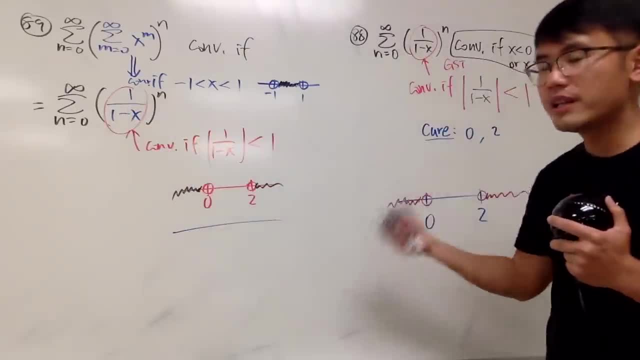 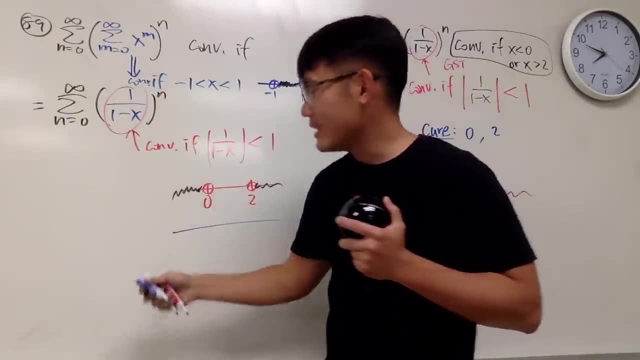 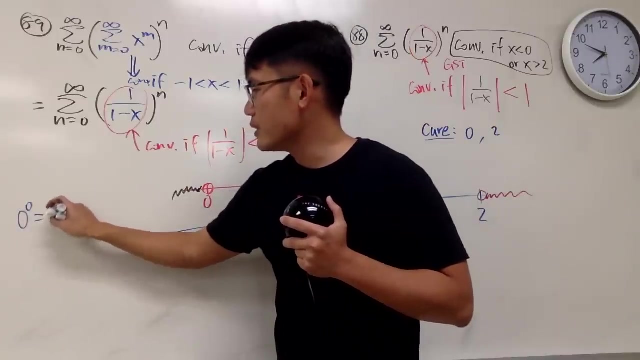 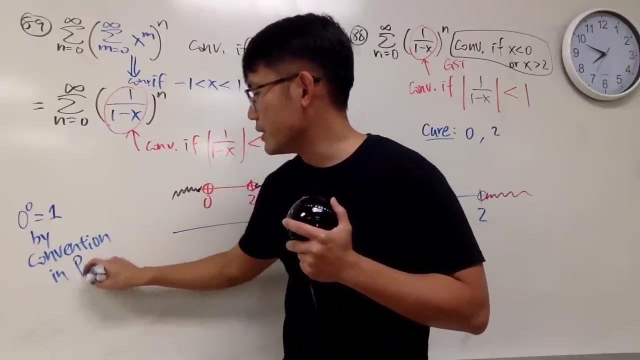 Two Conditions, So Perhaps I Will Just Put This Down. So This Is The One, Because I'll Just Tell You, Zero Equal To Zero Is. 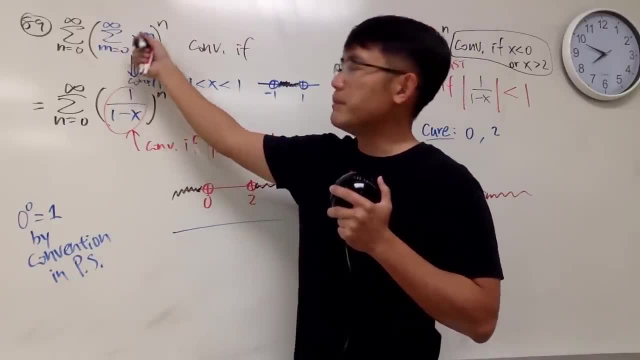 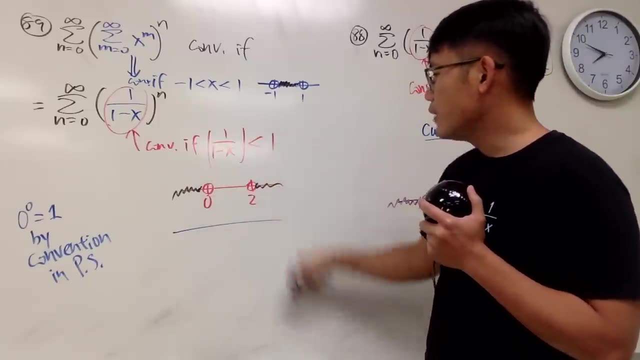 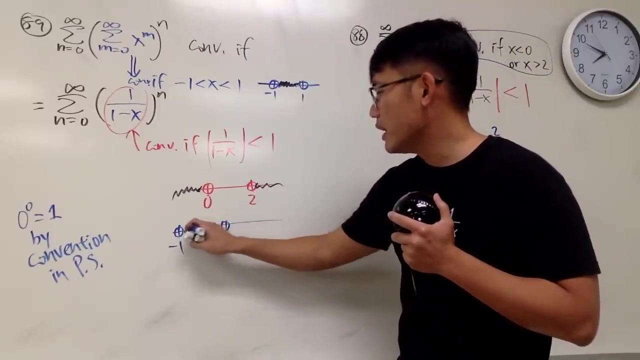 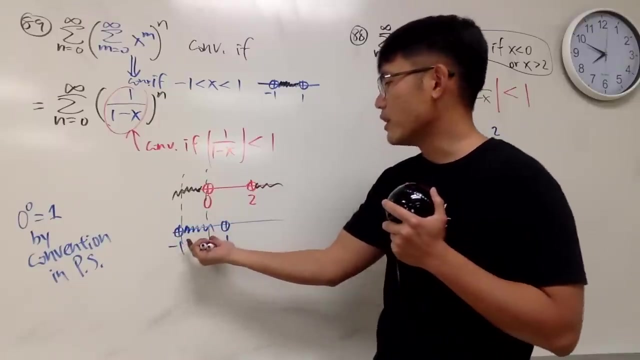 One By Convention In Power Series. So When X Is Zero And If You Put M Is Equal To, So Of Course You Look For The 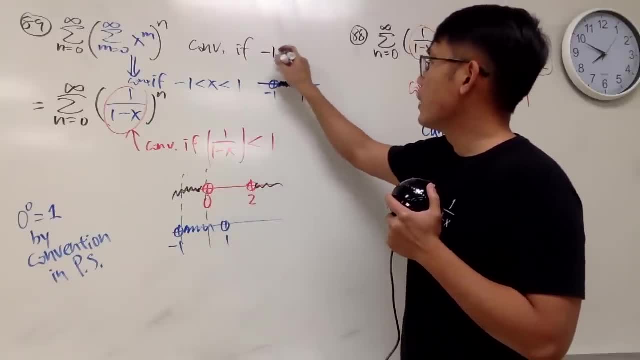 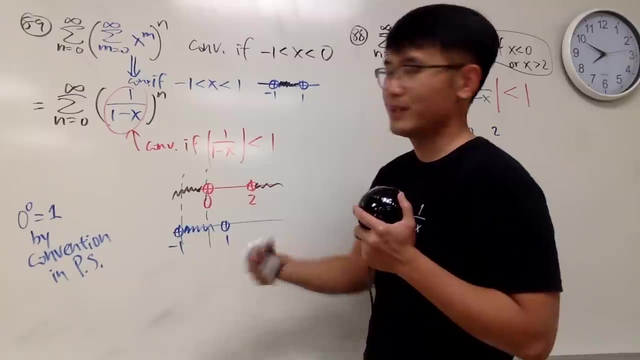 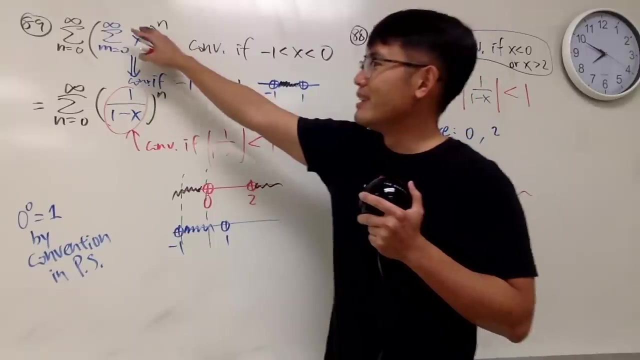 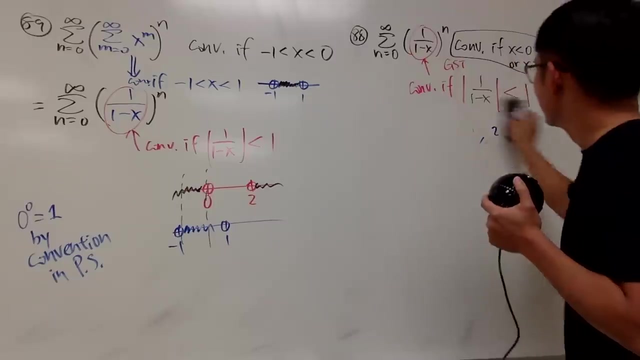 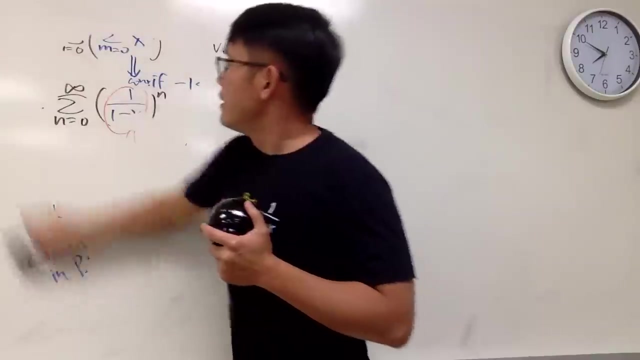 Common Area, The Comfort Interval Which Is From Zero To Negative One. That's The Idea. So It Converges Negative One X Zero. Very Cool. 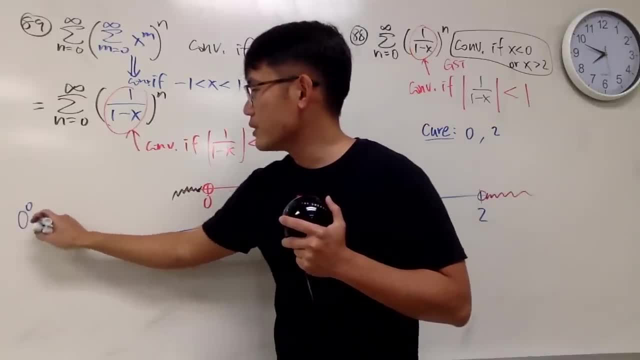 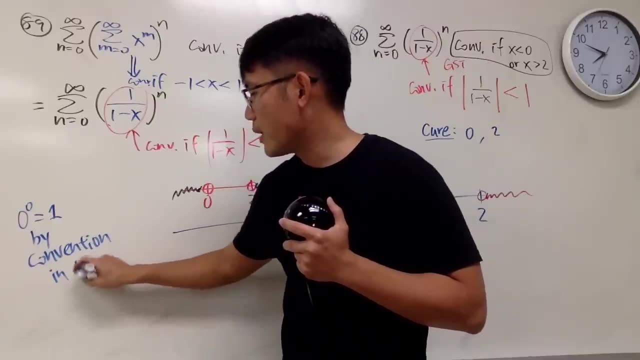 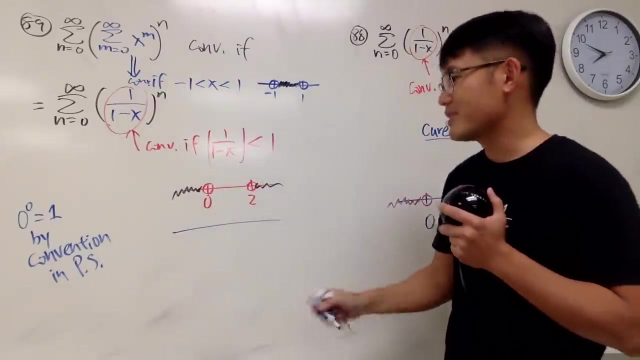 It's not a bunch of 0, because I'll just tell you, 0 equal to 0 is 1 by convention in power series. So when x is 0, and if you put m is equal to 0, then you actually get 1, so that's no good. So I can not plug. 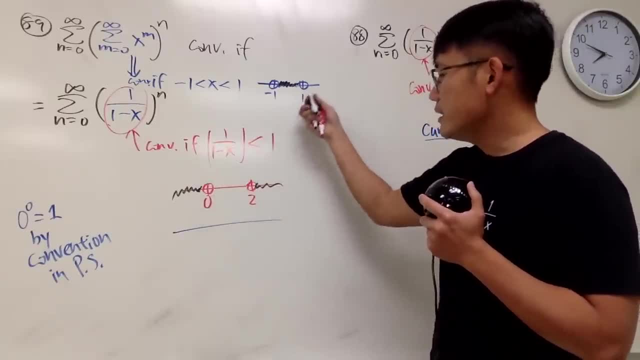 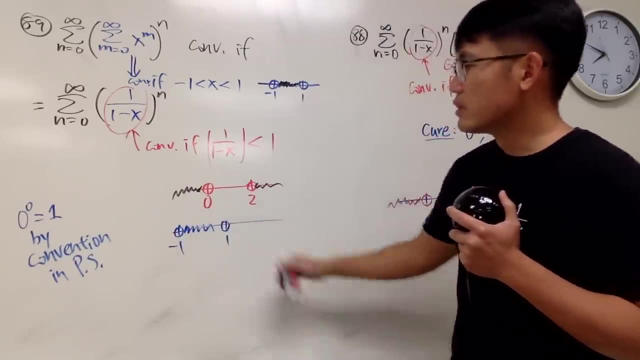 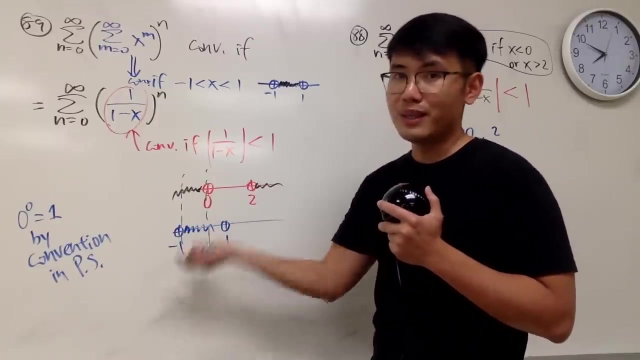 in. I can not have 0.. Anyway, if you look at this interval which is actually going from 1 to negative 1, open, open, and you want this point in between. So of course you look for the common area, the common interval, which is from 0 to negative 1.. That's the. 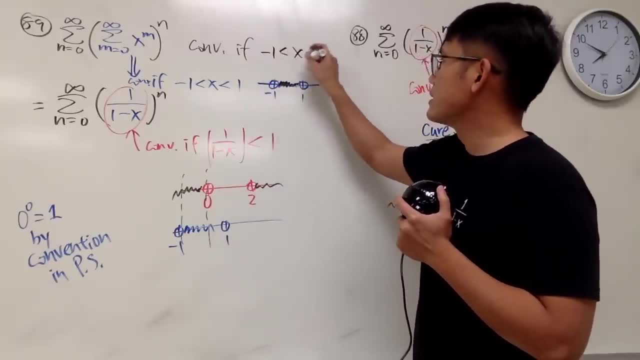 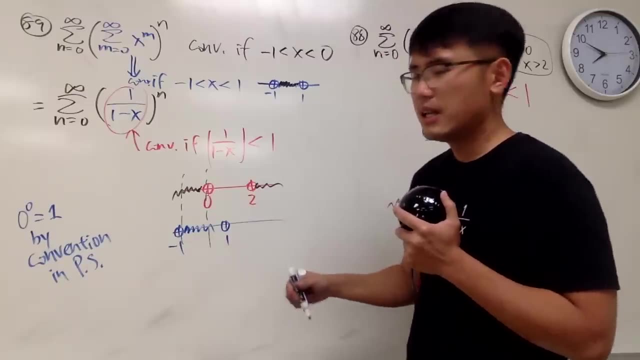 idea. So it converges negative 1, x, 0,. right That Again. do a quick check if you would like, but you know I will leave that to you guys. The truth is, if you plug in 1 half it's not going to work. 1 half, you get 2,. 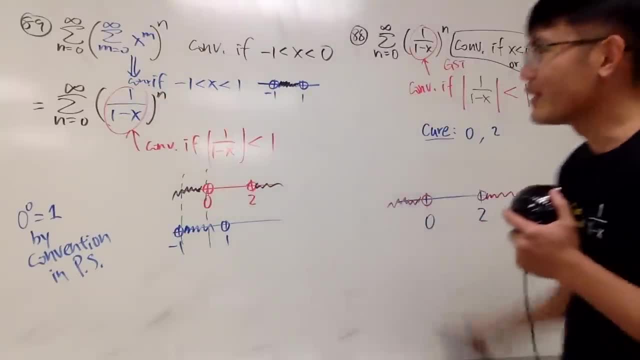 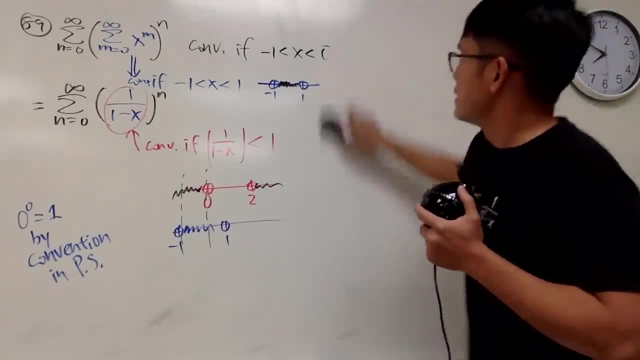 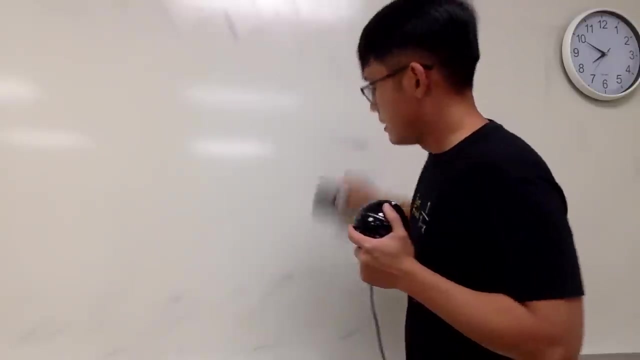 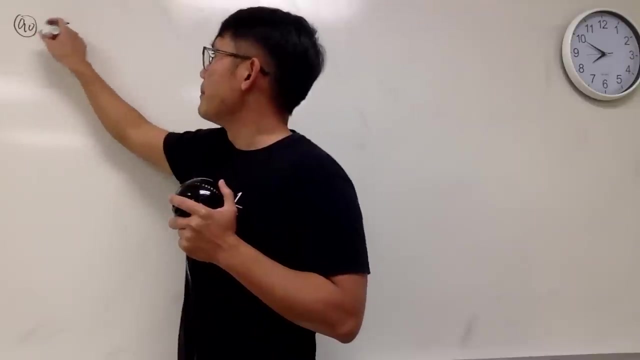 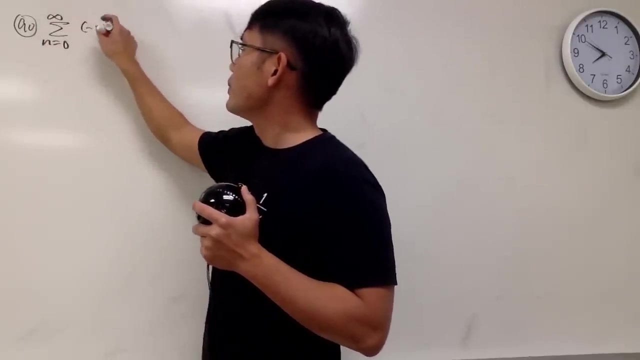 right, You get 2, and then 2 to n. no, no, no, no, no. So that's it Very cool, huh. Number 90,. right here, The sum as n goes from 0 to infinity negative, 1 to the n over. 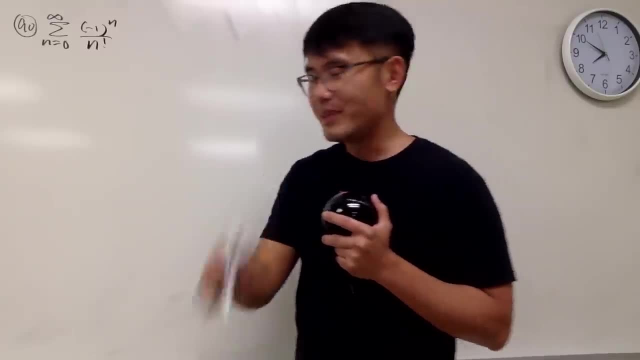 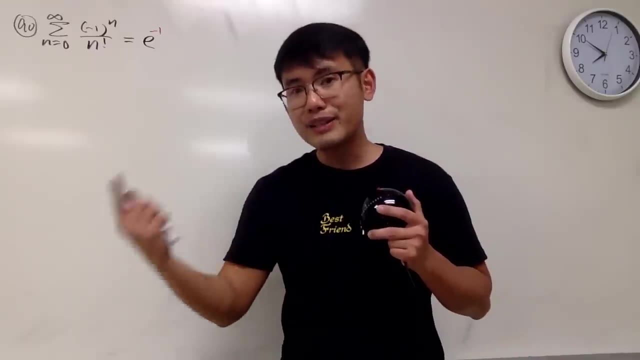 n factorial. This right here. let me tell you guys what the answer is. It's just e to the negative 1 power. Why? Because you have to know your other friends as well. So I will just write this down for you guys and I'll tell you guys the deal. 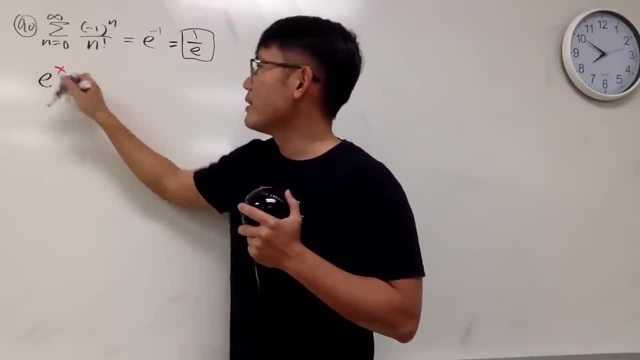 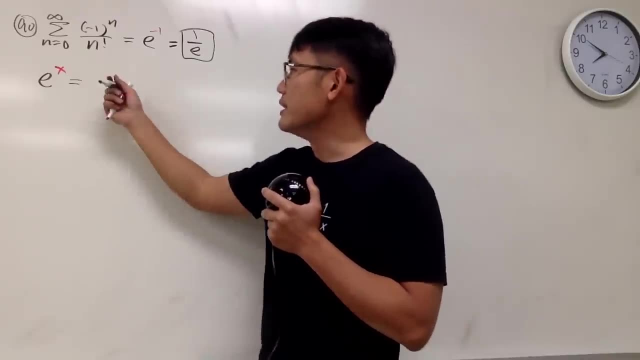 So here's the deal: When we have e to the x power- and in this video I'm not really working on the power series, I just want to test out the convergence and all that- But the truth is this: right here it's actually the sum as n goes from 0 to infinity, x to 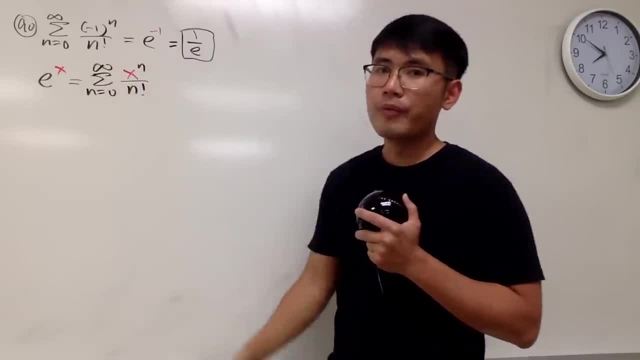 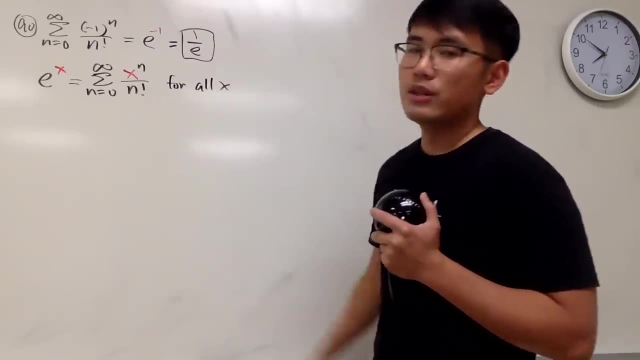 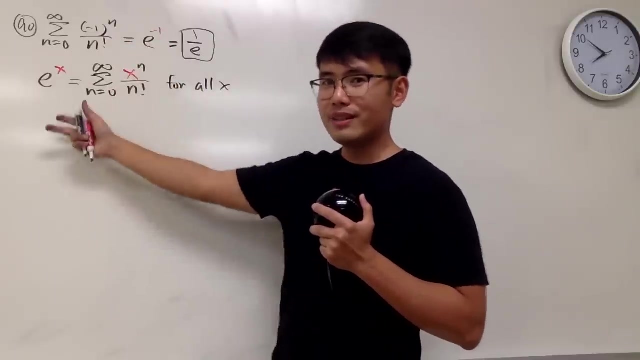 the nth power over n factorial. And this, right here, is true for all n, I mean for all x value. You can plug in whatever x and it will converge. As you can see, right here, we're just plugging in negative 1. So you plug in negative 1. So you have e to the 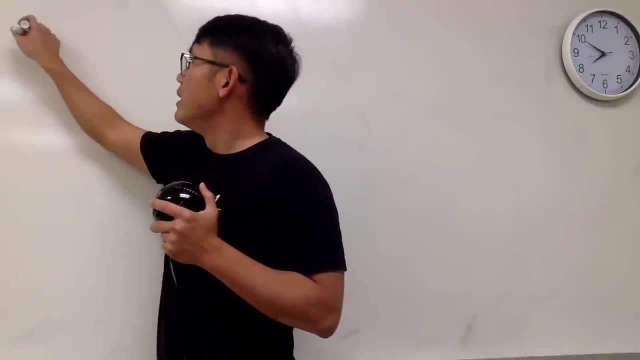 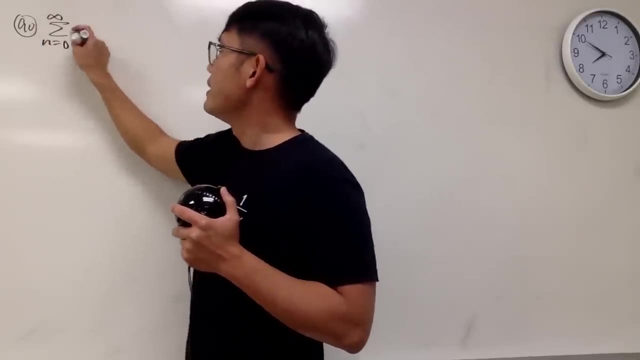 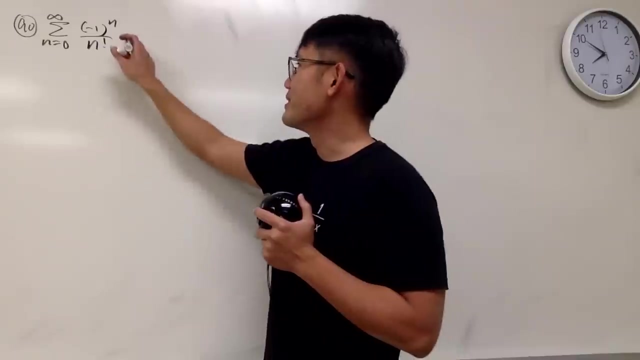 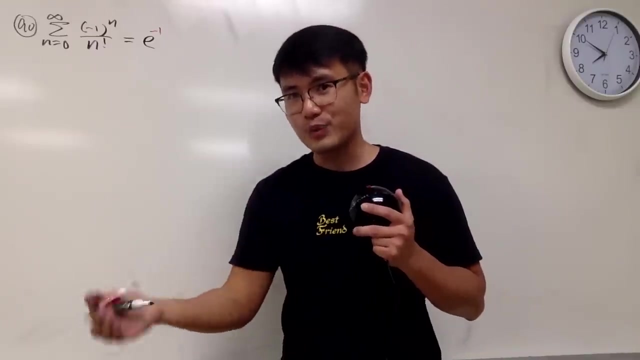 Number Ninety. Right Here. The Sum As N Goes From Zero To Infinity Negative One. This Right Here. Let Me Tell You Guess What? The 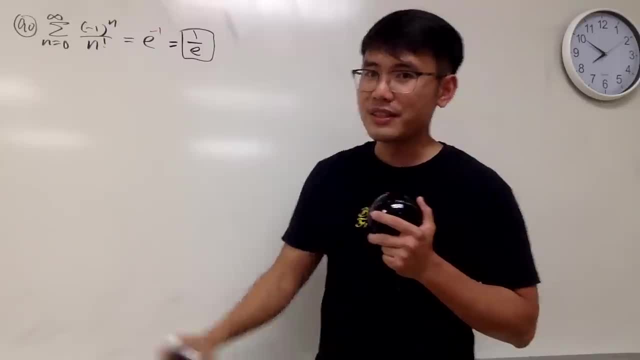 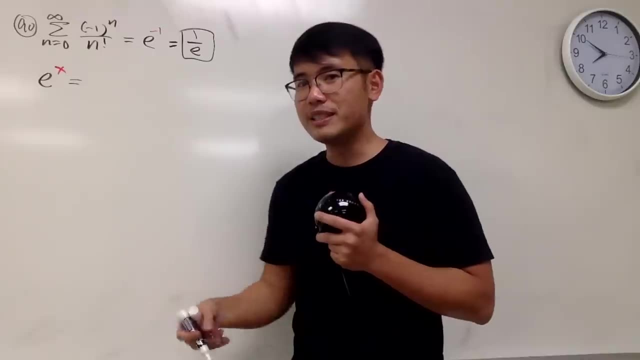 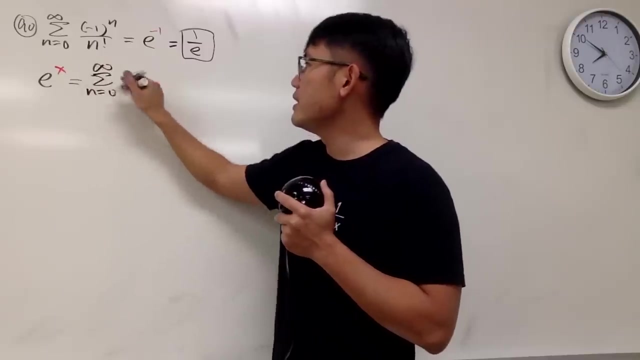 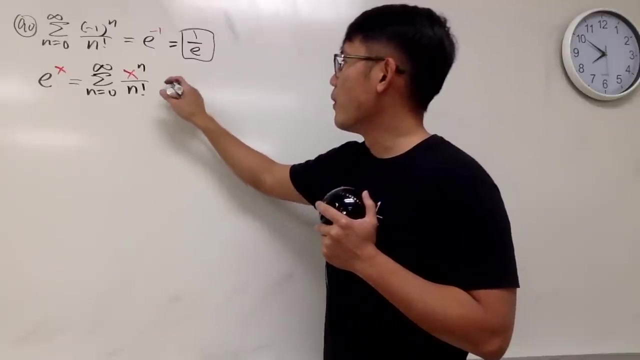 Answer Is Just E To The Negative One Power. Why? Because You Have To Know Your Other Friends. X To The N Power Over N Factorial. 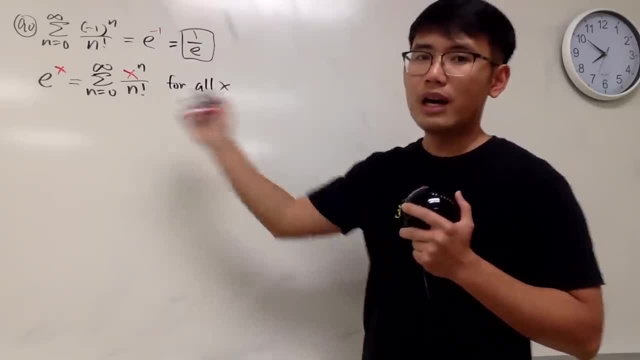 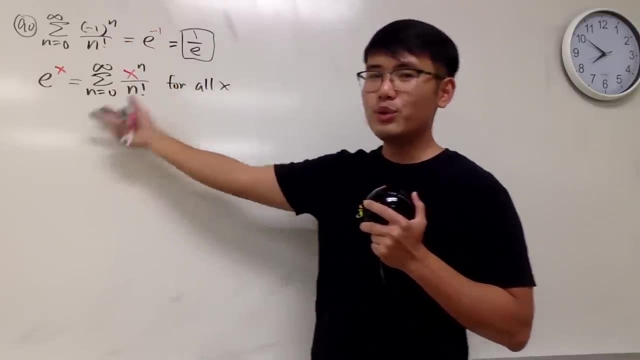 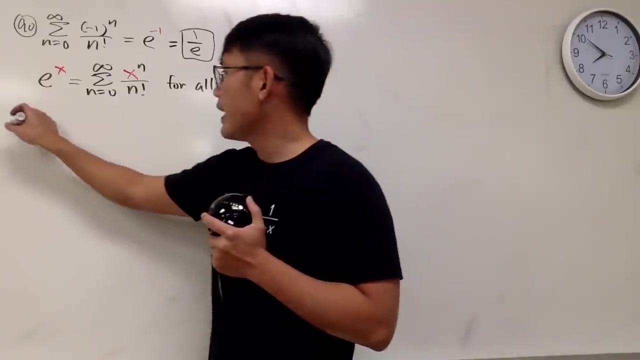 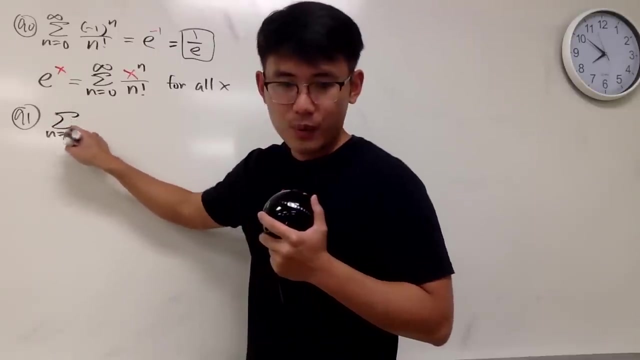 And This, Right Here, Is True For All N. I Mean For All X Value. You Can Plug In Whatever X The Sum As N Goes. 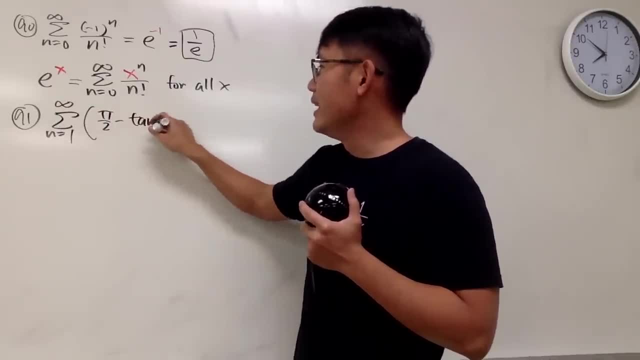 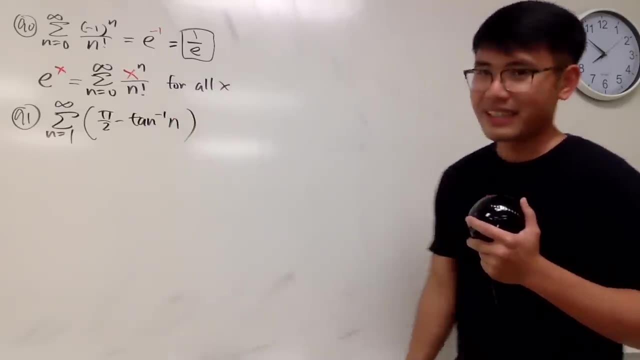 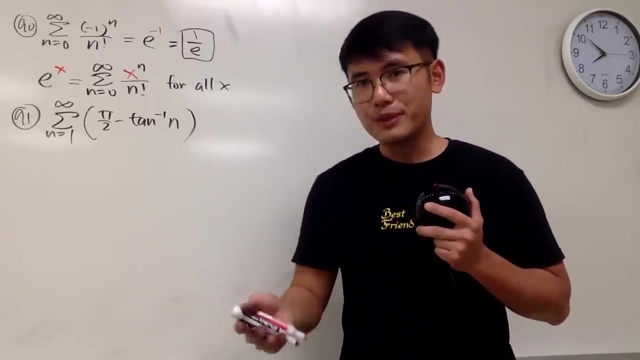 From One To Infinity, And Here We Have Pi Over Two Minus The Inverse Tangent Of N, Right Here. So This, Right Here You. 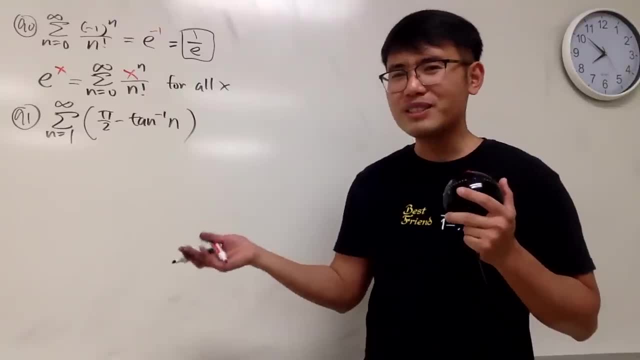 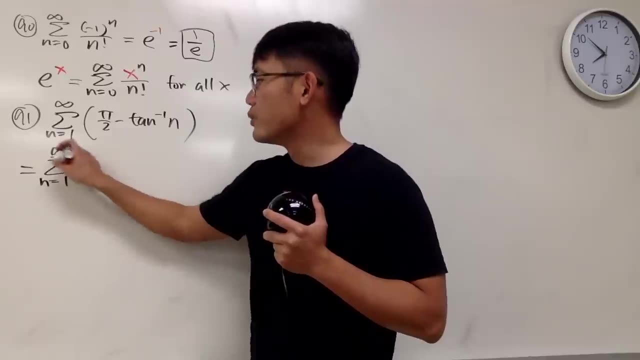 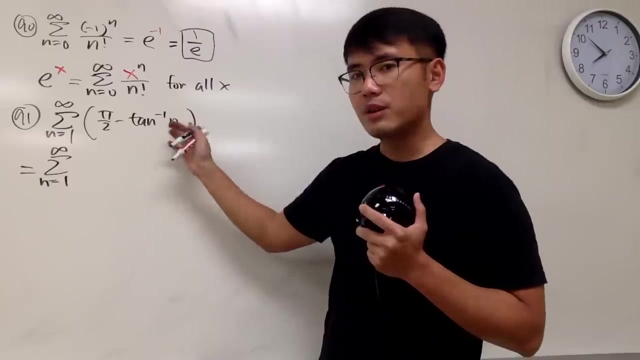 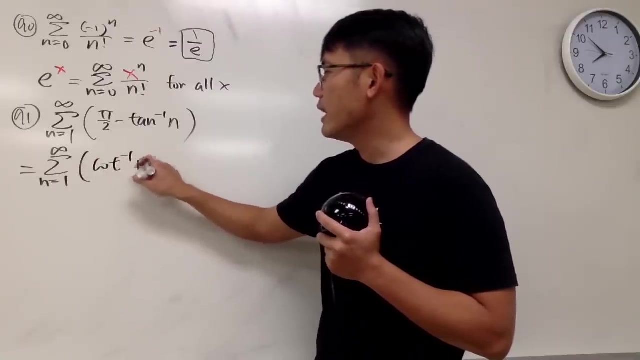 Can See And Hard To See What Kind Of Things We Can Use To Compare This With Right. So Now Let Me Show You The Good. 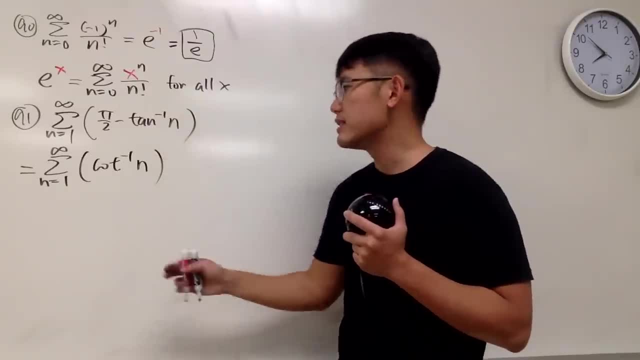 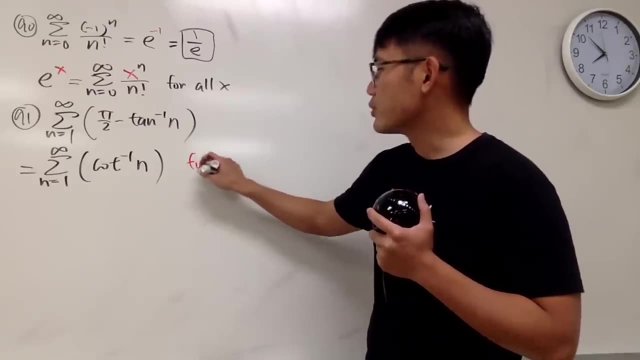 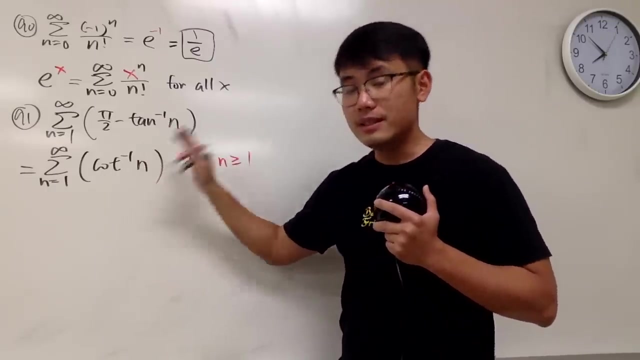 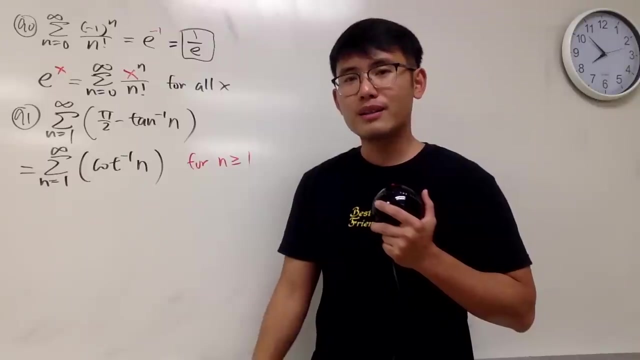 Thing Is That, In The Sense That Because Co Tangent Might Be Discontinuous And All That Stuff, So Notice This Right Here Is Actually True. 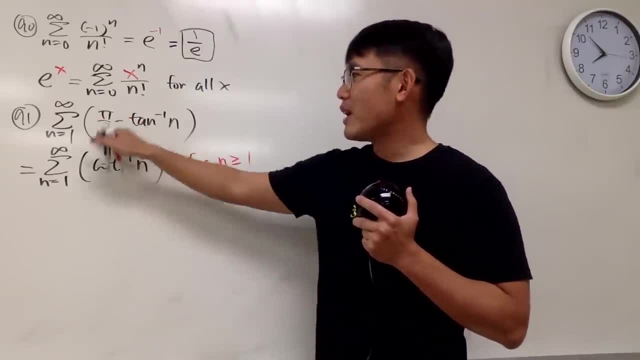 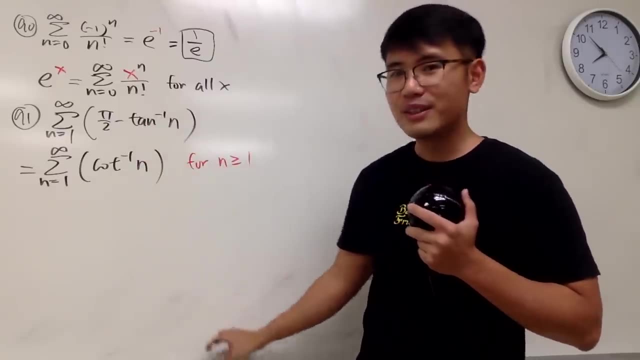 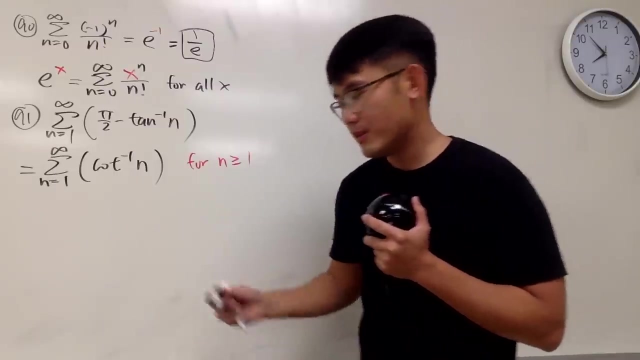 For N Greater Than Equal To One Co Tangent. Just That's The Idea. This Is Really Dirty To Realize. My Hands Still Dirty, But. 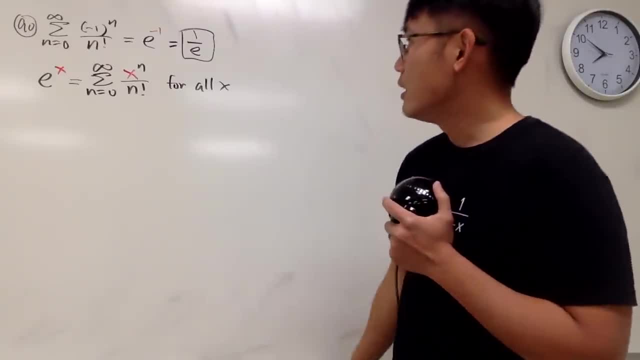 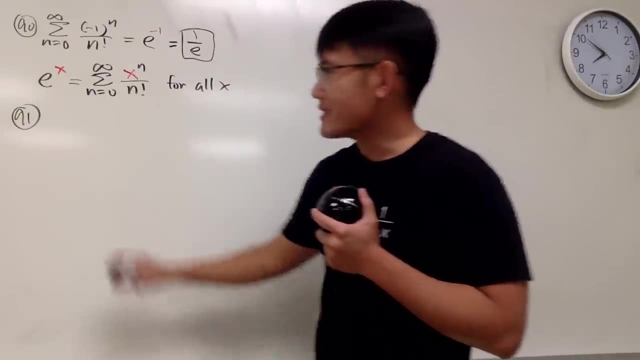 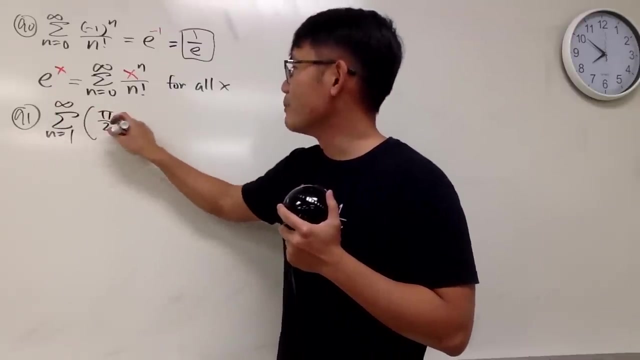 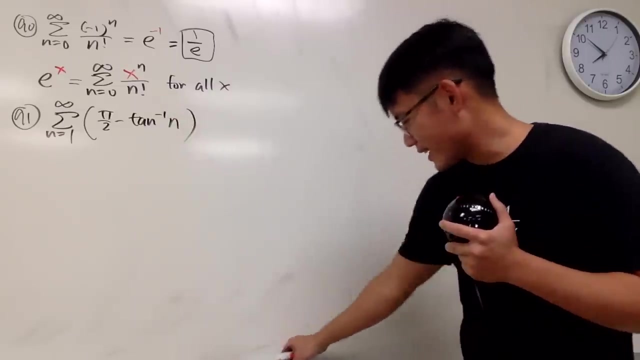 negative 1, and we are done. That's it. 1 over e. That's it Now, 91.. Oh my god. Nine more questions. The sum as n goes from 1 to infinity. And here we have pi over 2 minus the inverse tangent of n, right here. So this, right here you. 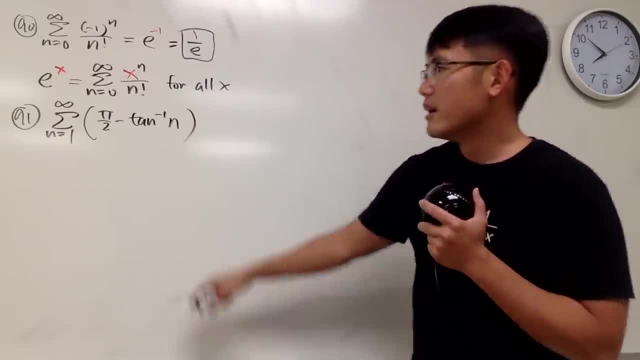 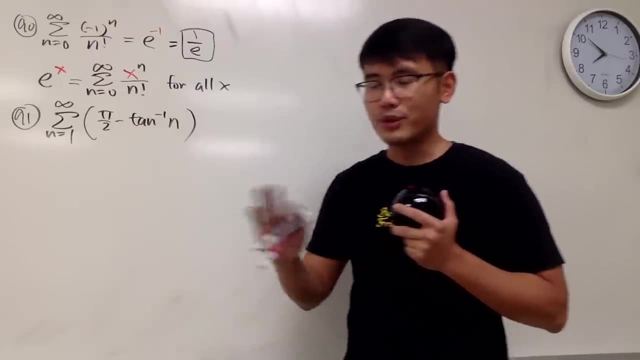 guys might not like it too much. First of all, if n goes to infinity, inverse tangent approaches pi over 2. So we have pi over 2 minus pi over 2.. So this right here, actually we can use the test for divergence. 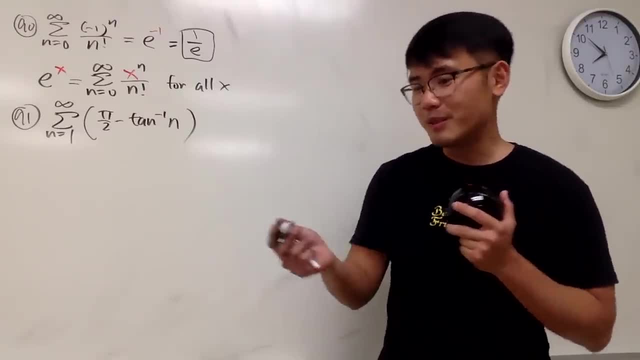 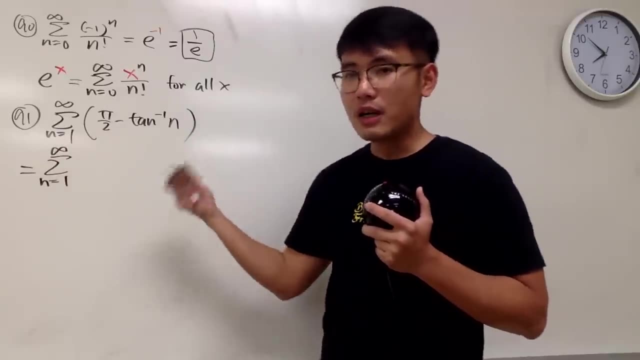 And it's hard to see what kind of things we can use to compare this with right. So now let me show you. The good thing is that when we have pi over 2 minus the inverse whatever trig function, pi over 2 minus. 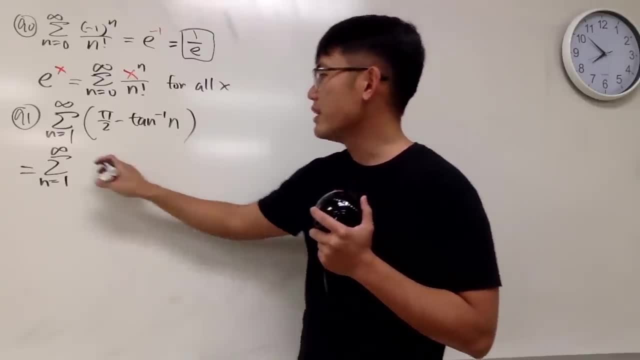 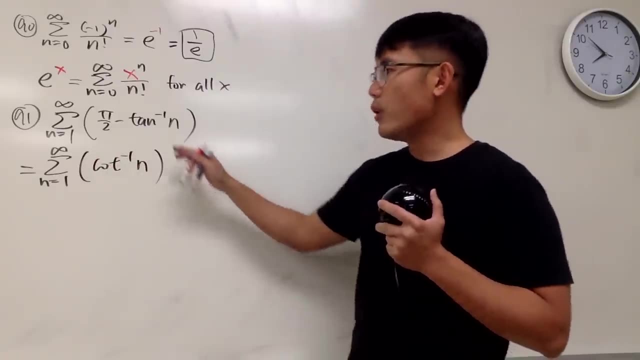 Oh, it's the inverse to the inverse of whatever. it's just the coversion of that. This right here is actually just the coversion, which is the cotangent of n. like this, And some people are not going to like this too much in the sense that because cotangent might 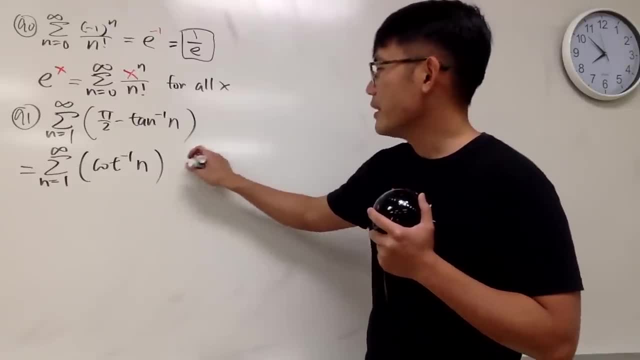 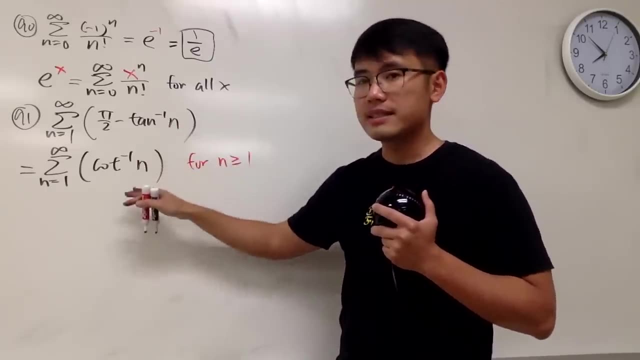 be say discontinuous and all that stuff. so notice this right here is actually true for n greater than or equal to 1.. If you grab this and that, if you replace the n with x, they will all be true, Right. 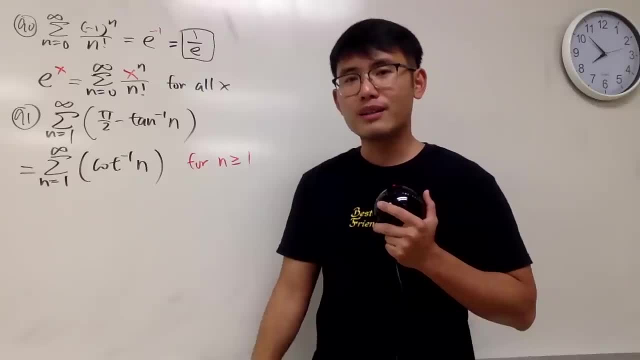 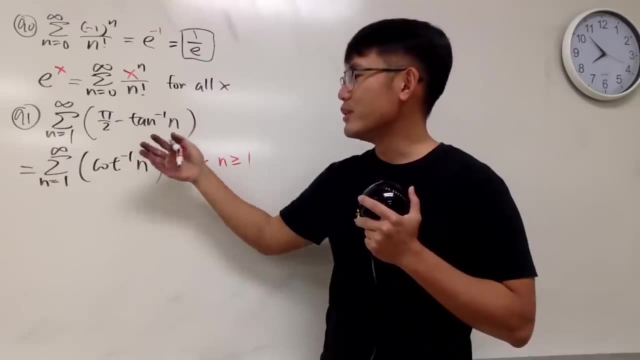 Pi over 2 minus arc sine, you get arc cosine. Yeah, you just get the co-version of that. So pi over 2 minus arc tangent, you get arc cotangent. Just that's the idea. This is really dirty. 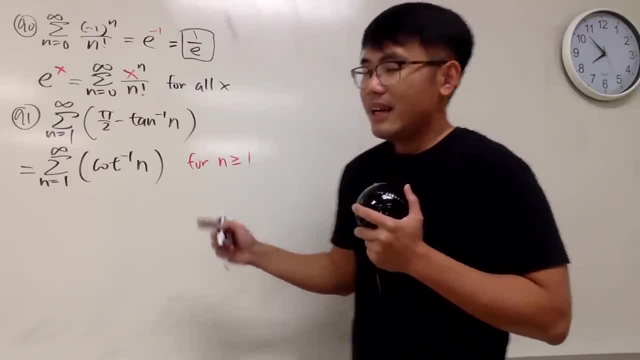 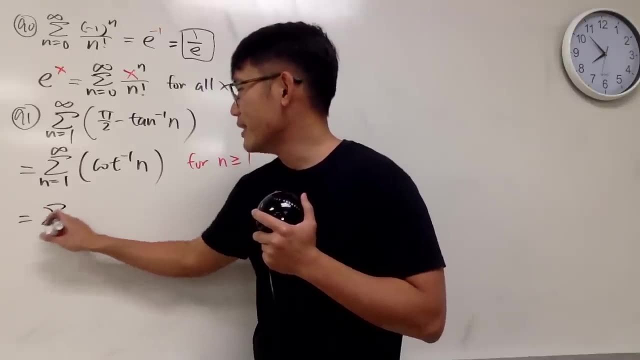 My hand is still dirty, but, oh well, I still don't know how to deal with this too much. Well, another thing you have to know is this: right here is, in fact: n is equal to 1 to infinity. 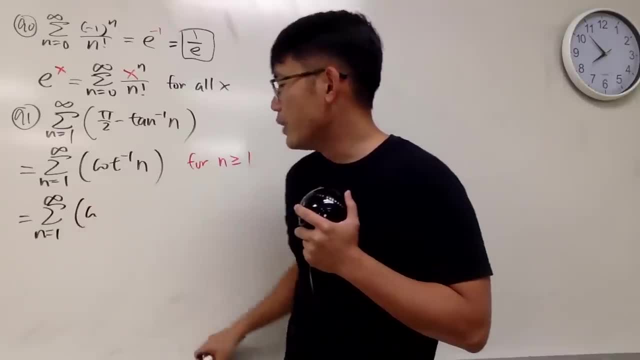 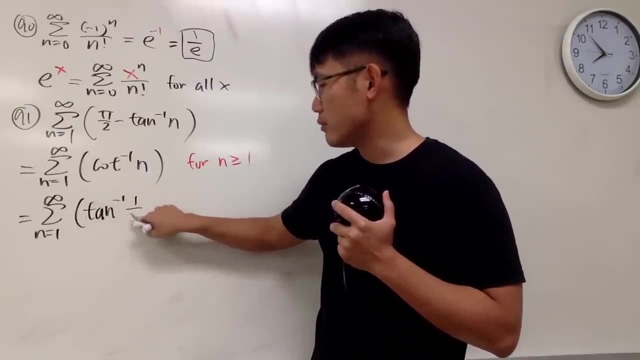 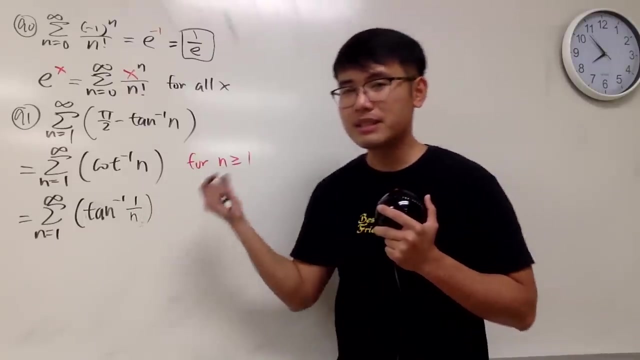 The arc cotangent of n is actually the same as regular inverse tangent, So it's the arc tangent inverse tangent And the input is actually 1 over n. And this is true for positive inputs, for positive inputs. For the negative inputs there might be some like debate. 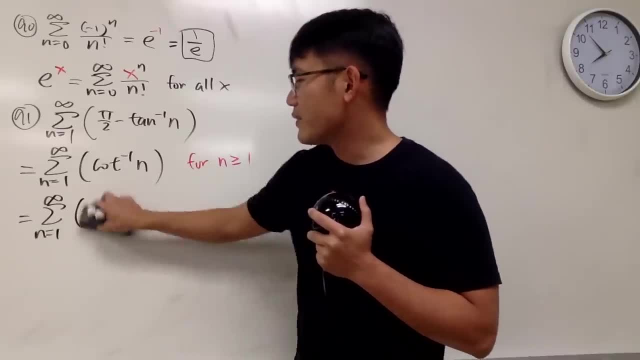 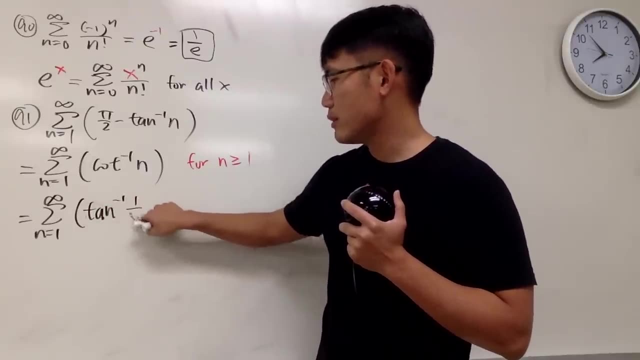 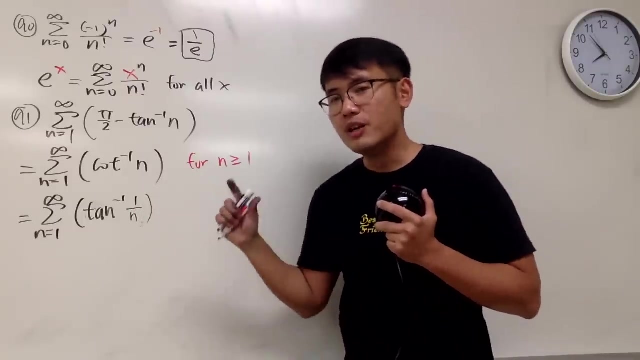 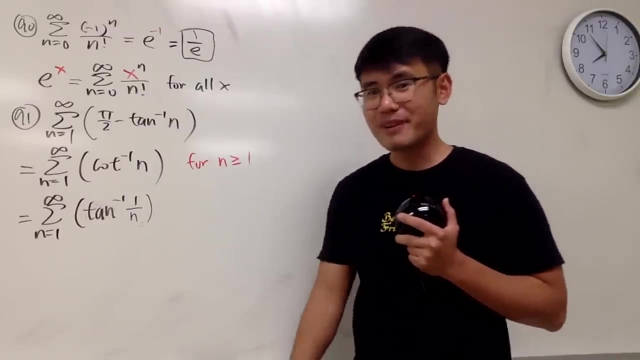 Oh Well, I Still Don't Know How To Deal With This Too. This Is True For Positive Inputs, For Positive Inputs, For The Negative Inputs. 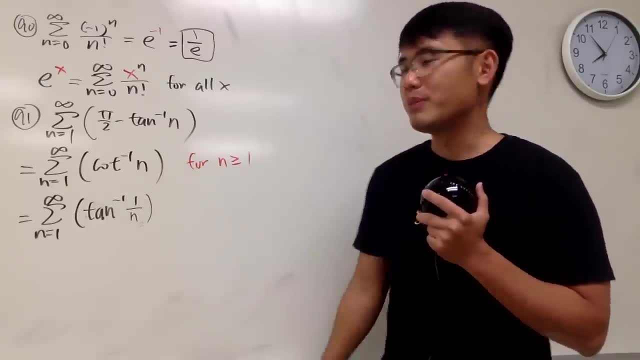 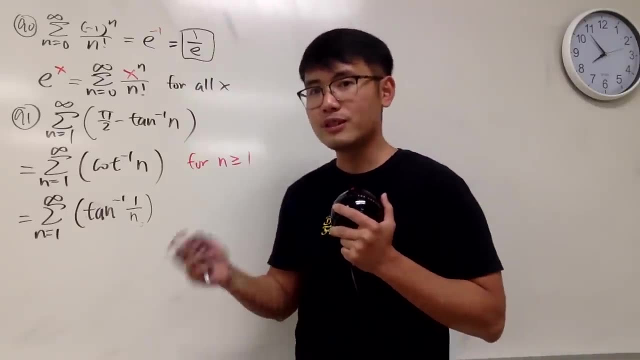 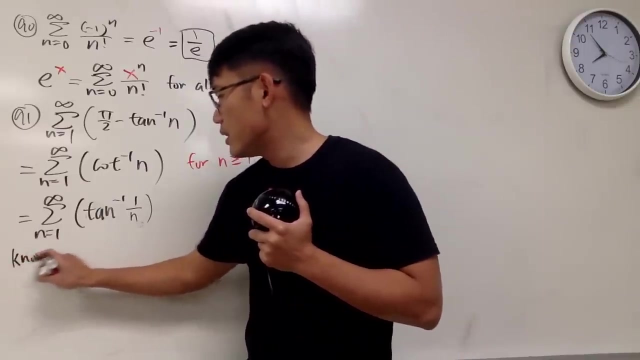 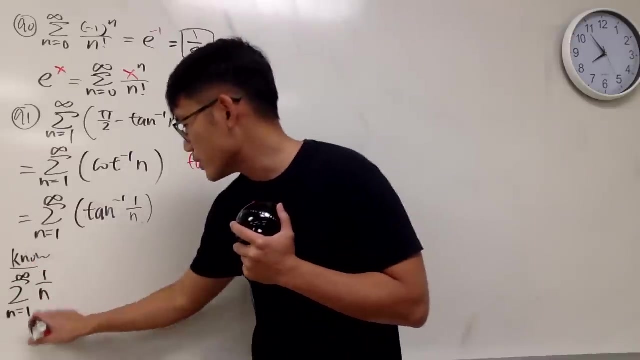 There Might Be Some Like A Debate, But For Positive Inputs We Are Good, Right If We Some As N Goes From One To Infinity One. 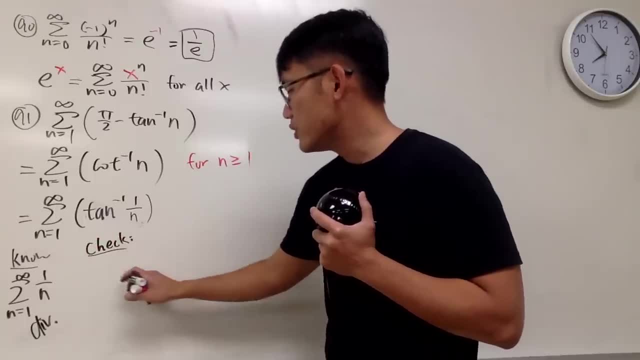 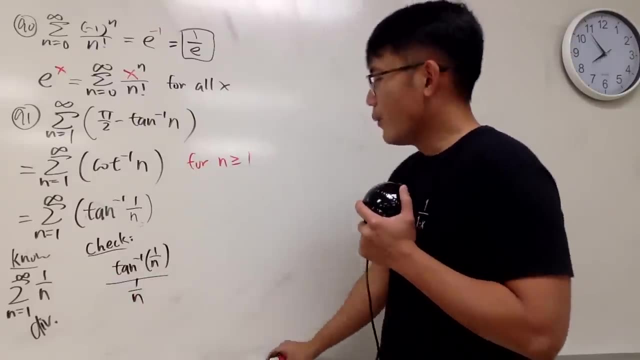 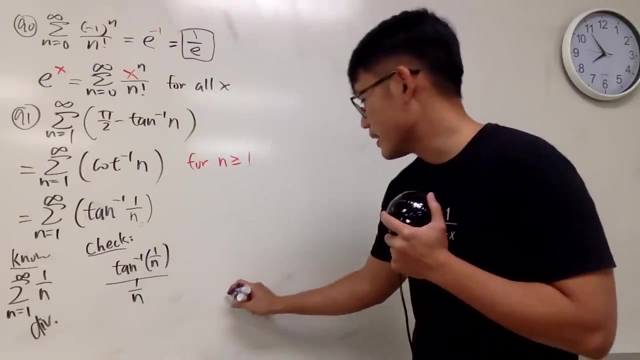 Over N. Let's Compare This With That, Because We See The One Over N. This Right Here Diverges One Over X, One Over X. 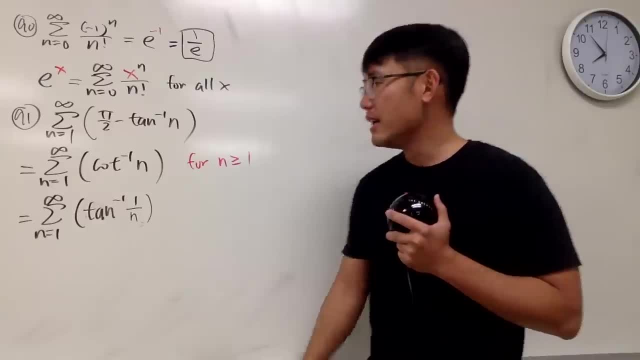 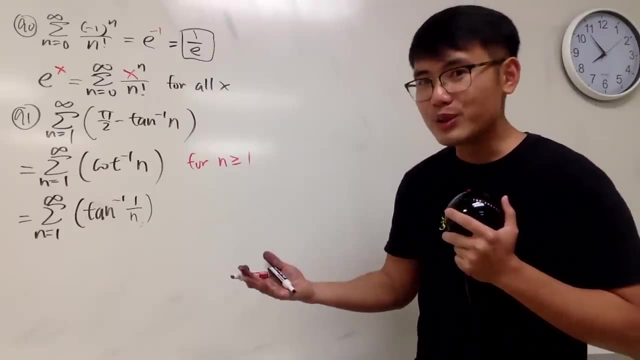 but for positive inputs we are good. If you want to know how to get that, leave a comment down below, I'll show you. But for this part I'll show you. You guys know the deal now. huh, We can actually just do what. 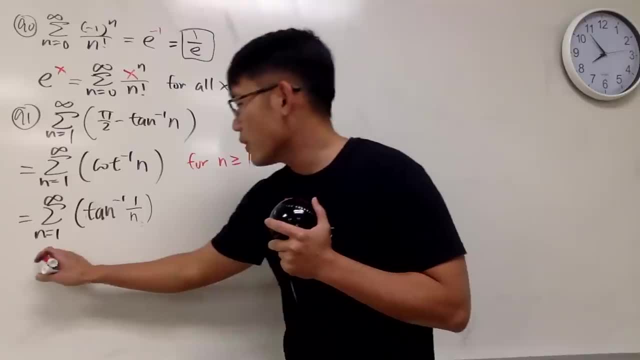 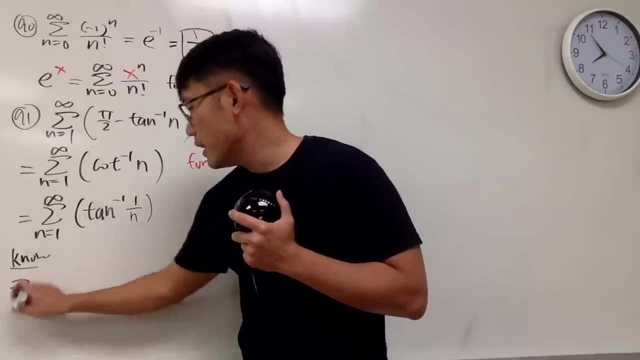 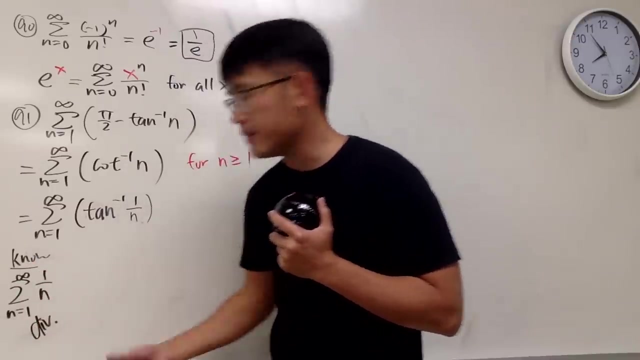 Yes, let's go ahead and just do the co-version test for that. So I know from here now the sum as n goes from 1 to infinity, 1 over n. let's compare this with that, because we see the 1 over n. 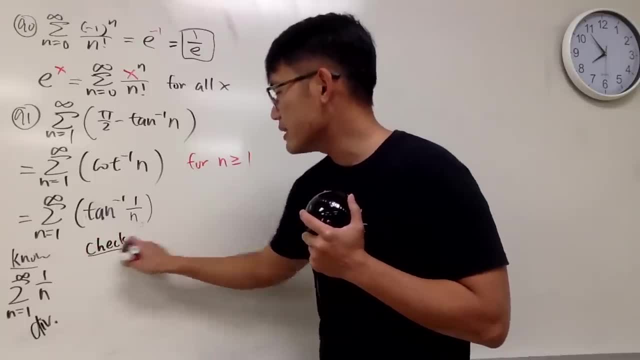 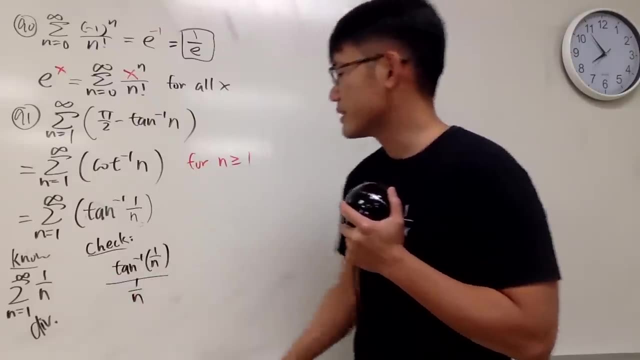 This right here diverges. and let's do the limit co-version test, Check the inverse tangent of 1 over n, n over 1 over n, like this. Well, let's just look at the x-version right here, real quick. 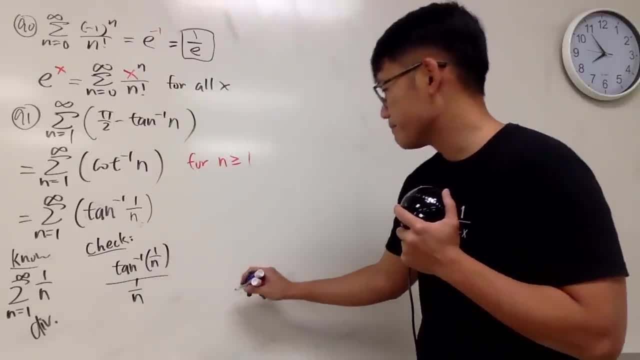 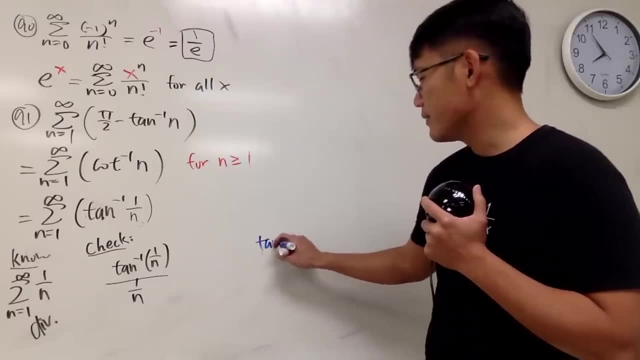 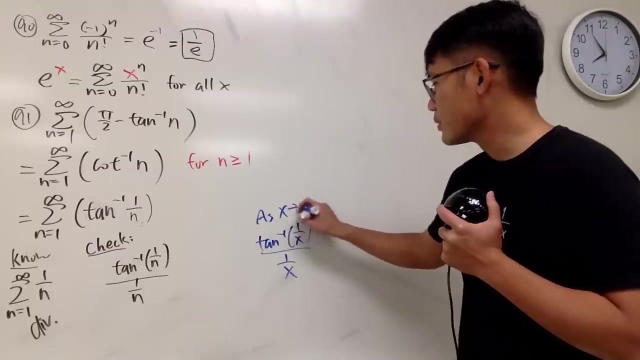 So I'll put this down. okay, So I'll just write this down. Yeah, inverse tangent of 1 over x, 1 over x, right? So this is when s x goes to infinity. All right, so differentiate everybody. 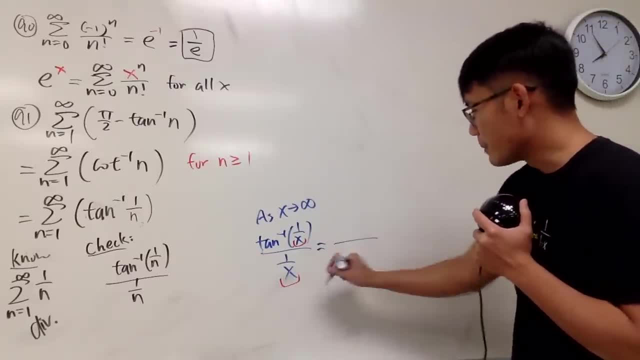 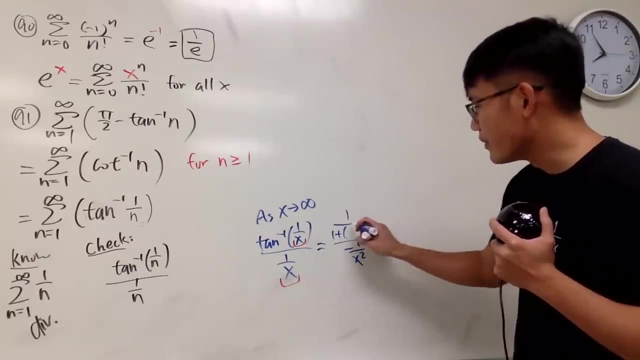 Here is the difference We get: the derivative on the bottom is negative: 1 over x squared. The derivative of this guy is 1 over 1, plus parentheses of the things inside the squared, because that's the inverse tangent, and the chain do says multiply by this, which is negative: 1 over x squared. 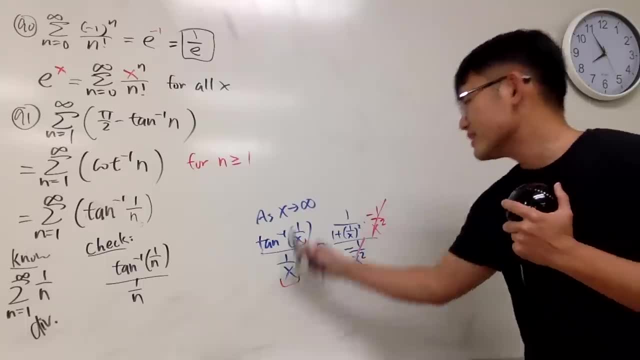 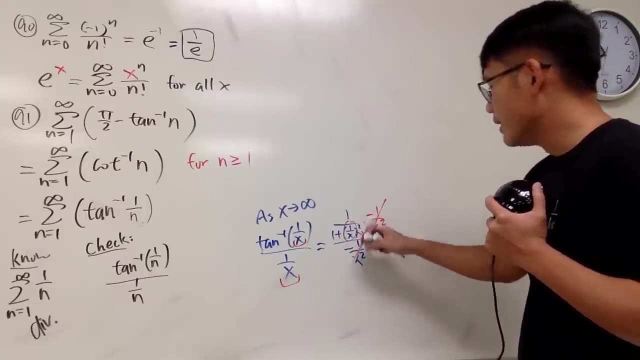 So cancel this out. Very nice, huh. And then, as x goes to infinity, this is 0.. So we get this going to 0, and we just have 1.. Very nice, So we'll come back here and we'll just write this down. 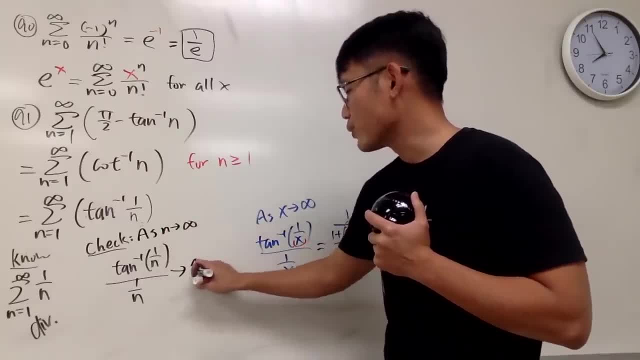 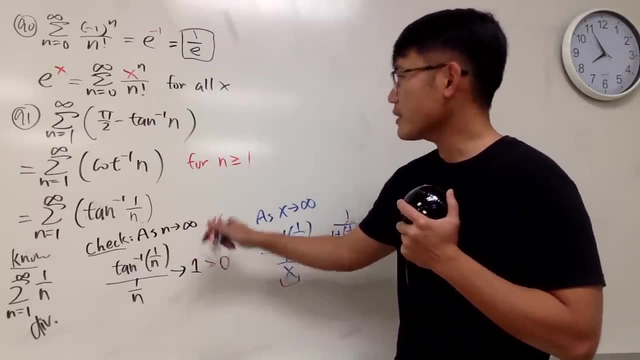 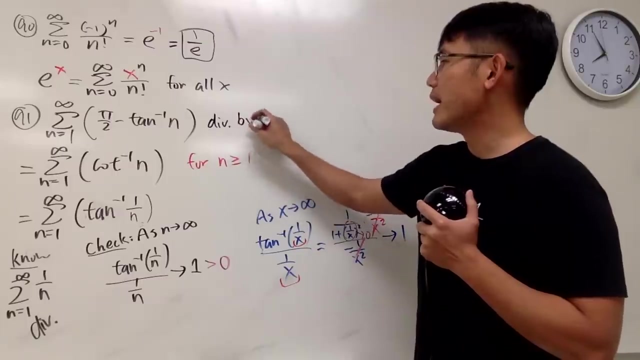 As n goes to infinity, this right here actually goes to 1.. This is a limit completion test. 1 helps because it's greater than 0. So we know this right here actually have the same conclusion as that one, which also diverges by the limit completion test. 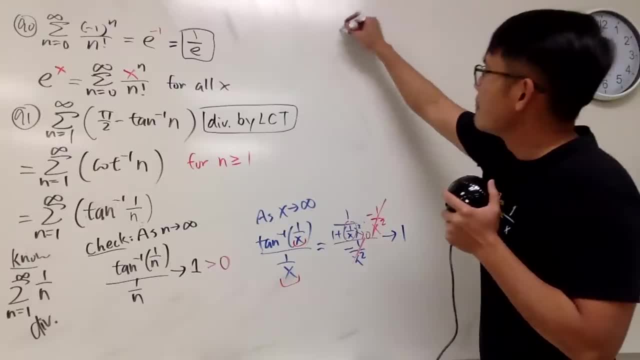 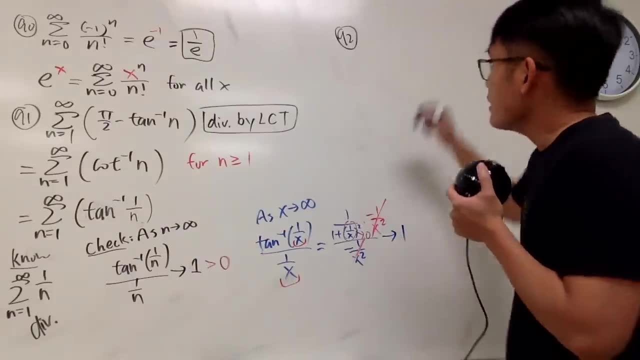 Aha, just like that. Okay, Now number 90. 2.. Okay, I cannot go home by 9.. I cannot go home by 8 o'clock, All right, Anyway, next one, Sine, okay. 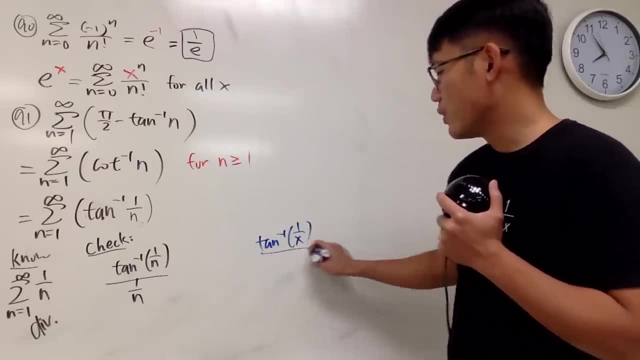 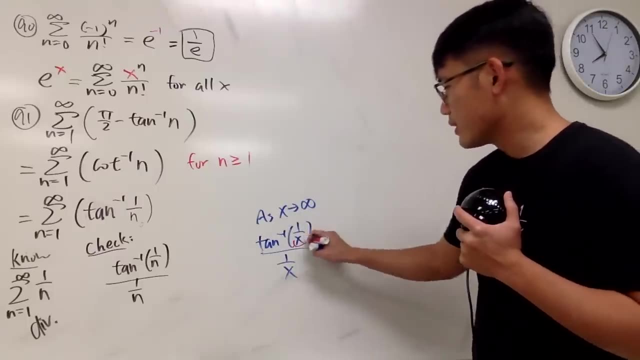 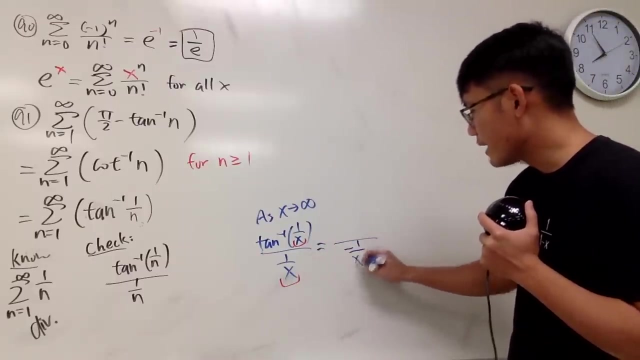 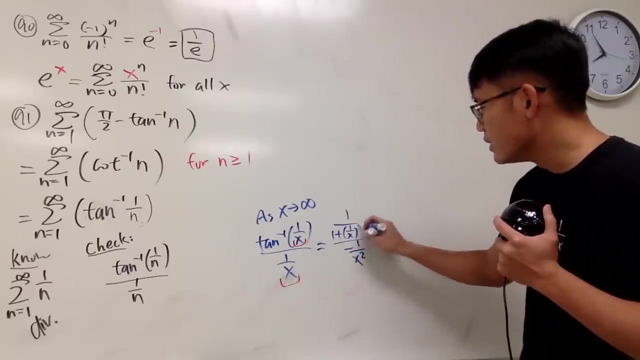 Right. So This Is When As X Goes To Infinity. All Right, So Differentiate Everybody. Here Is The Deal: We Get The Derivative Of The. 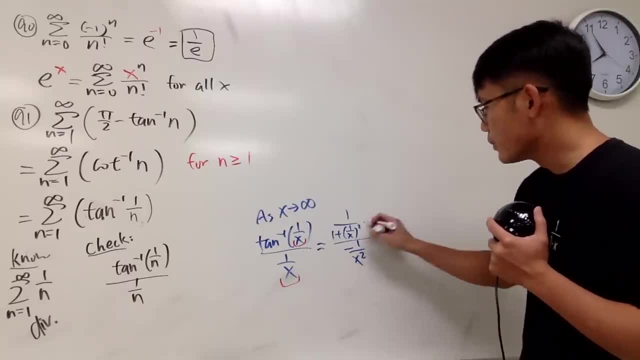 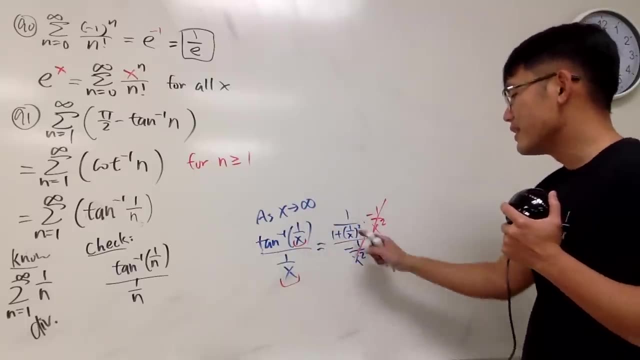 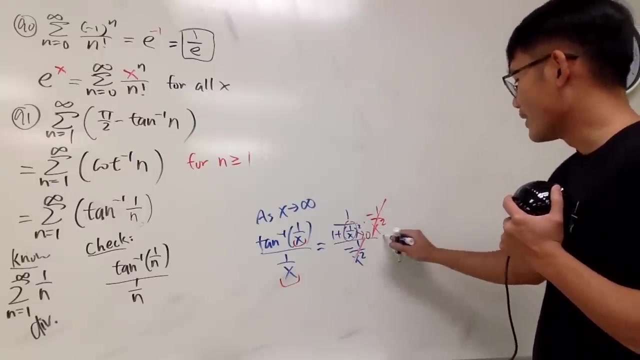 Things Inside The Square, Because That's The Inverse Tangent And The Chain Do Says: Multiply By This, Which Is Negative. One Over X Square. 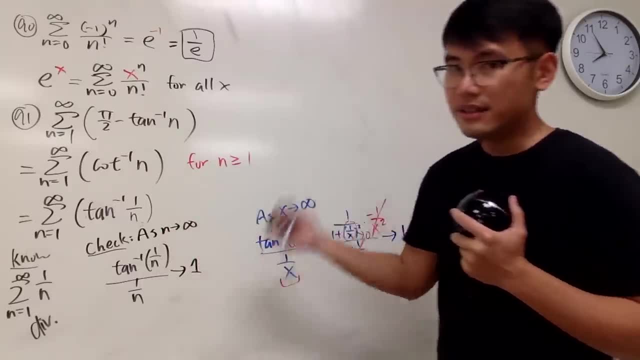 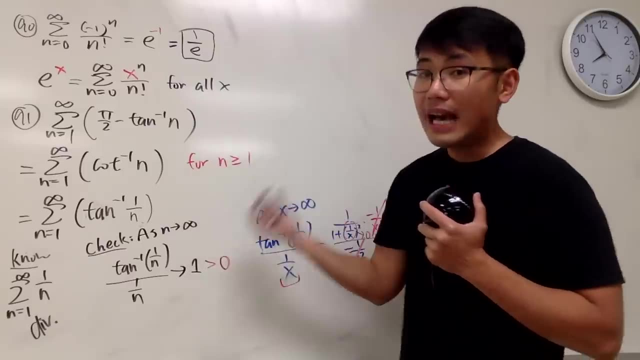 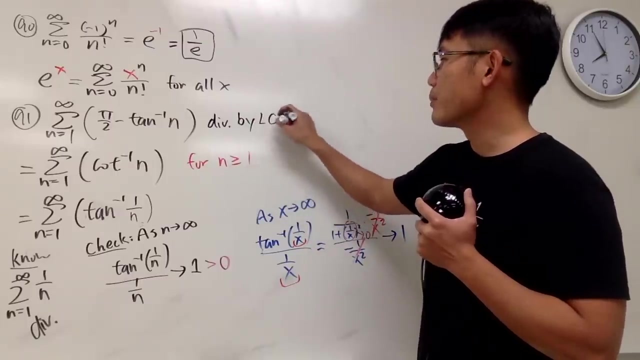 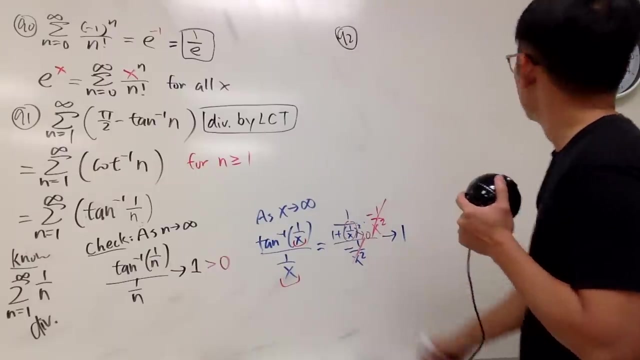 So Cancel. This Is A Limit Completion Test. One Helps Because Is Greater Than Zero, So We Know This Right Here. Actually Have The Same Conclusion. 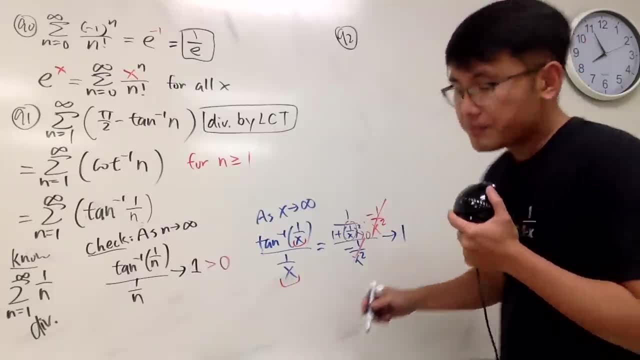 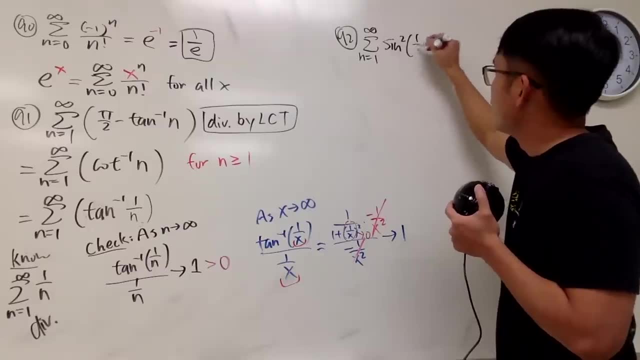 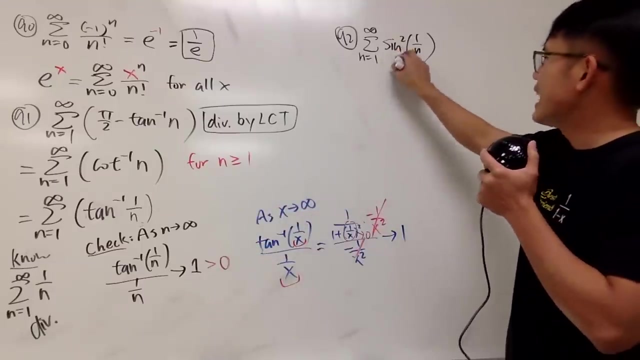 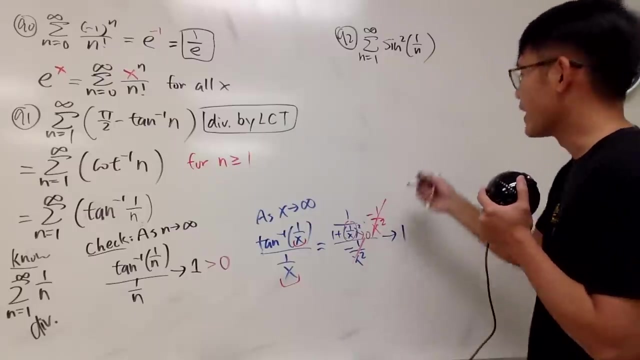 As That One Which Also Diverges Okay And Goes From One To Infinity Sign Square Of One Over N. Here You Might Want To Use. 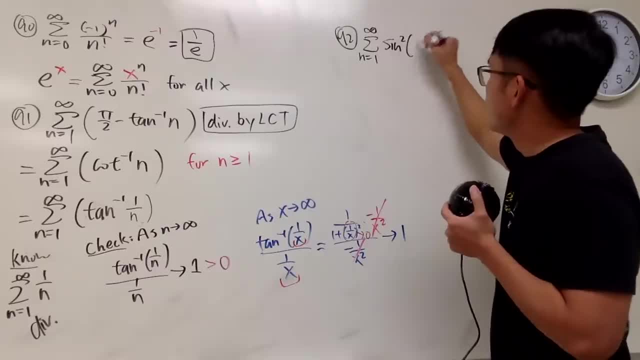 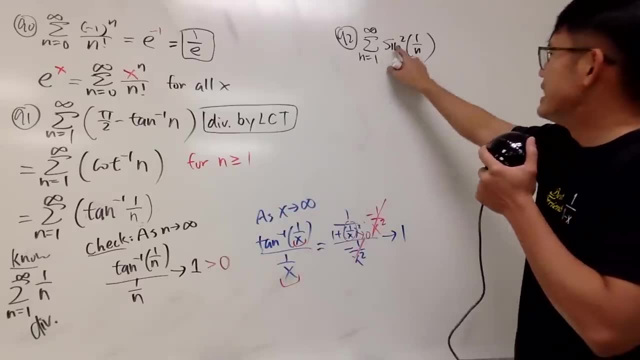 n goes from 1 to infinity. Sine squared of 1 over n. Hmm, Here you might want to use the 1 over n as well, but this is sine squared. The truth is, we actually have to use 1 over n squared. 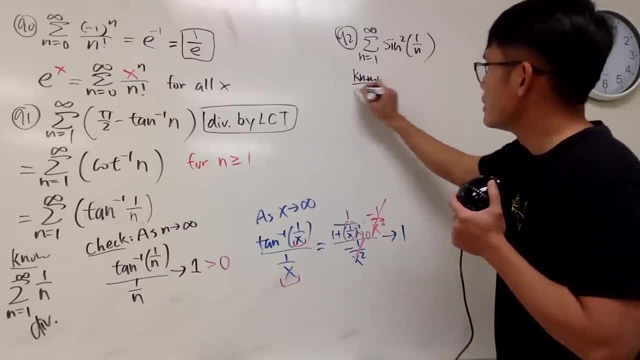 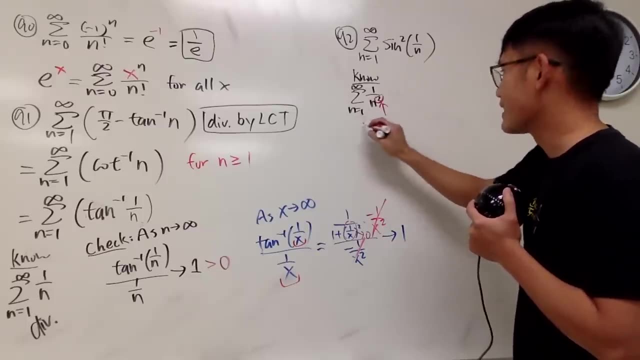 like the series for that. So let me show you. We actually know the sum, As n goes from 1 to infinity, of 1 over n. squared this right here. how many times have we used it? A lot, right. 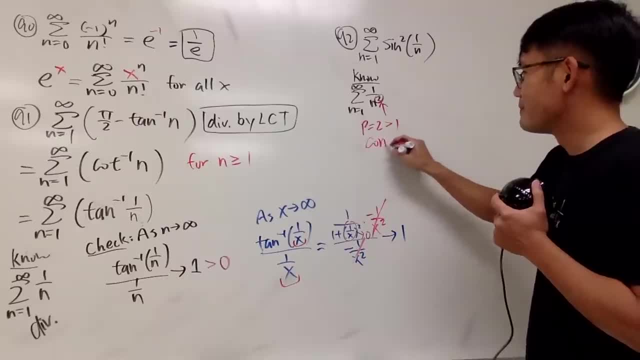 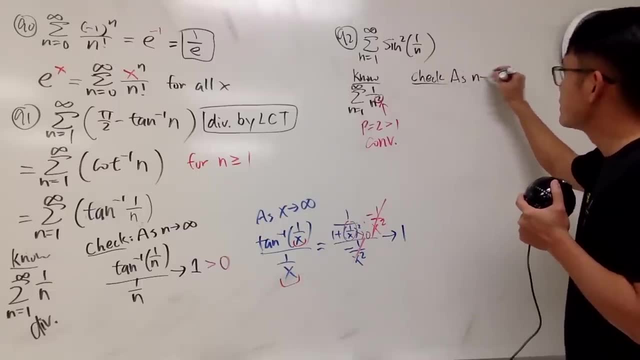 So better make sure that you get this right. This right here converges And then we are going to check S? n goes to infinity. This is not bad, because I hope we can use the best friend. What I mean? the? 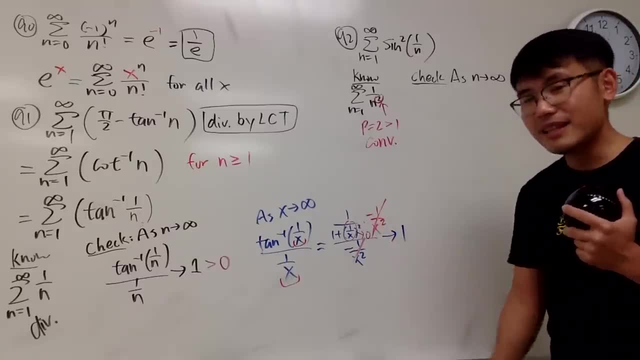 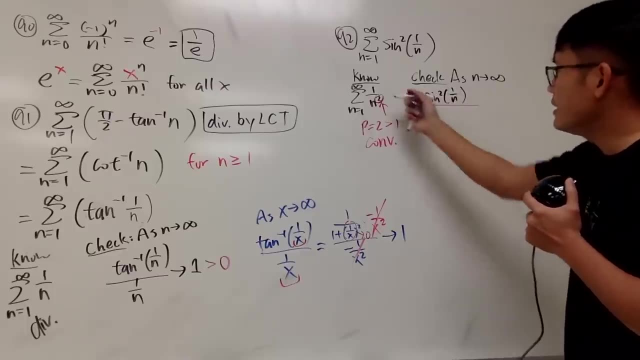 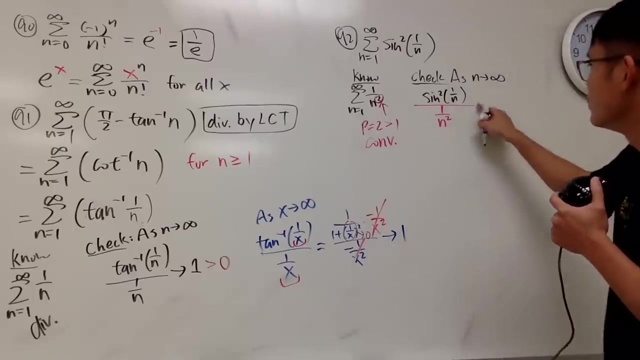 We can. We can actually use the limit. You will see. Put the 1 right here on the top, Sine squared of 1 over n, over this on the bottom. This is why we use 1 over n? squared, because, you know, sine squared is the same as saying: 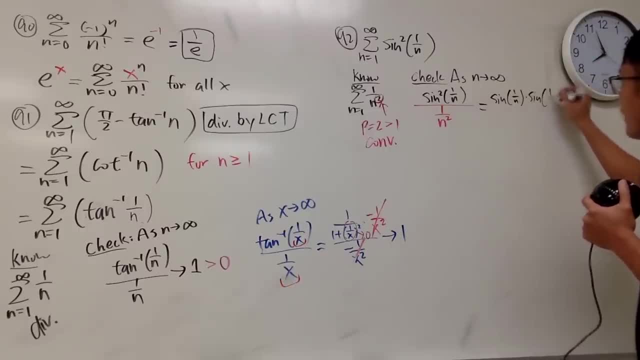 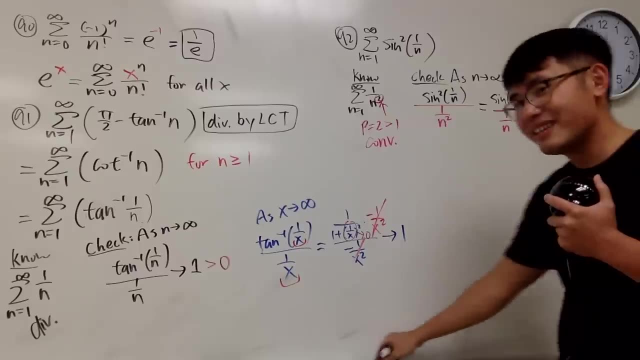 sine of 1 over n times sine of 1 over n, And of course I can write this as 1 over n times 1 over n, Everybody happy. And of course, if you want to really call the limit- I mean yeah, to call the limit- you can just say: 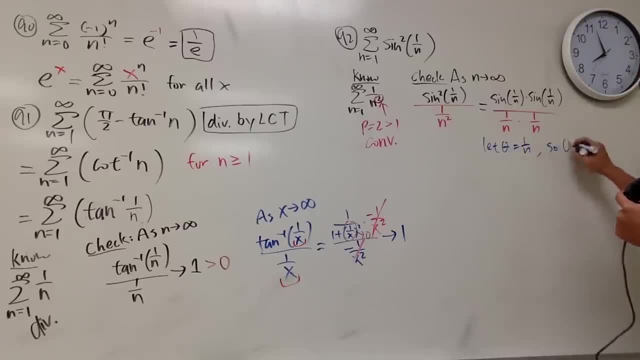 let theta equals 1 over n, So theta goes to 0.. And this right here becomes sine of theta, times sine of theta, And we have this divided by theta, divided by theta, And this right here approaches 1 and 1.. 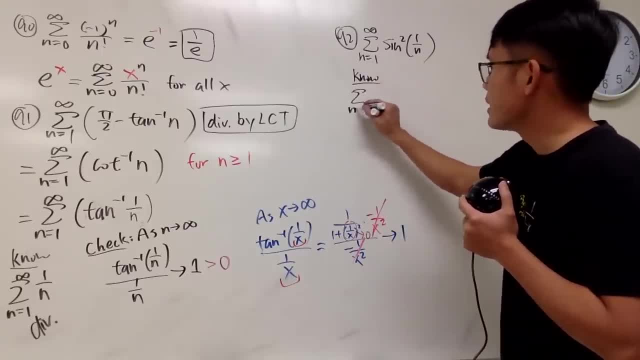 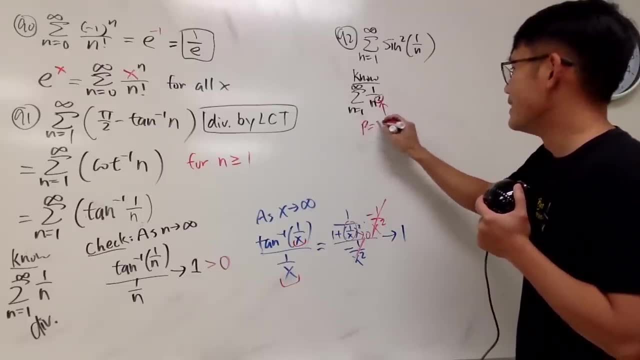 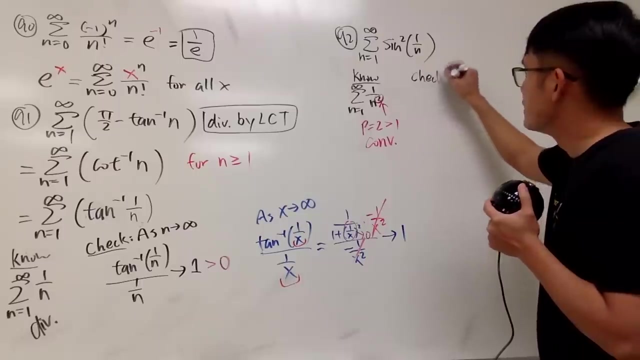 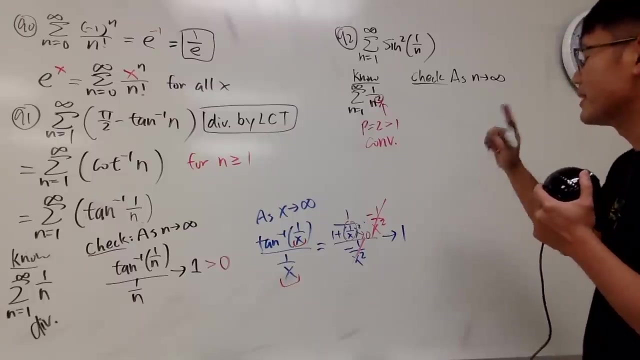 The One Over N As Well, But This Is Sign, So Better Make Sure That You Get This Right. This Right Here Converges And Then 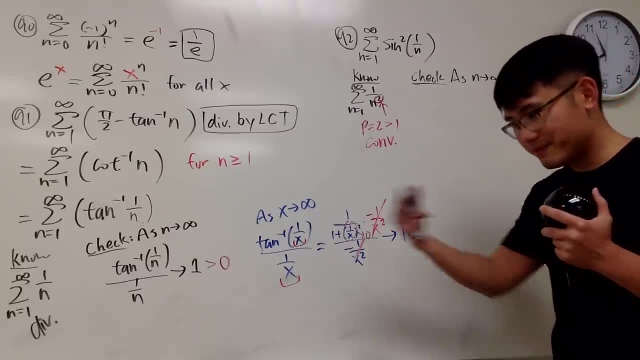 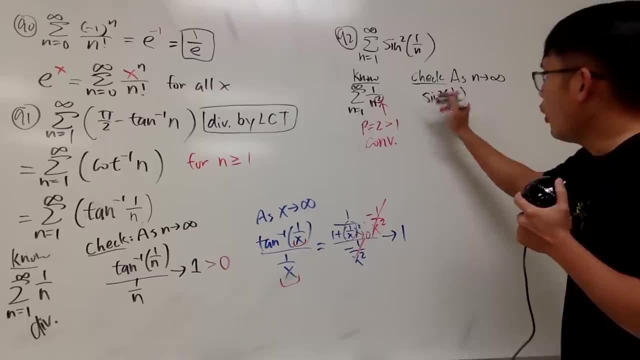 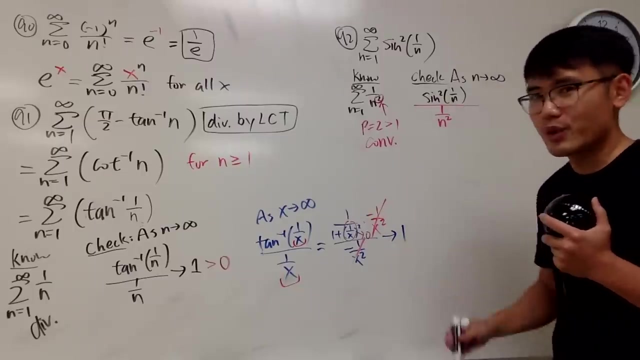 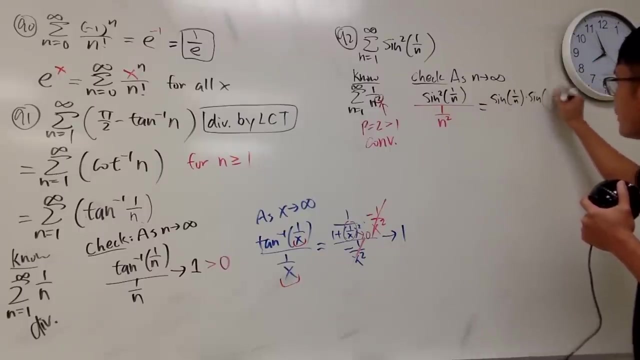 We Are Going To Check As N Goes To Infinity. This Is Not Bad. This Is Why We Use One Over N Square, Because You Know. 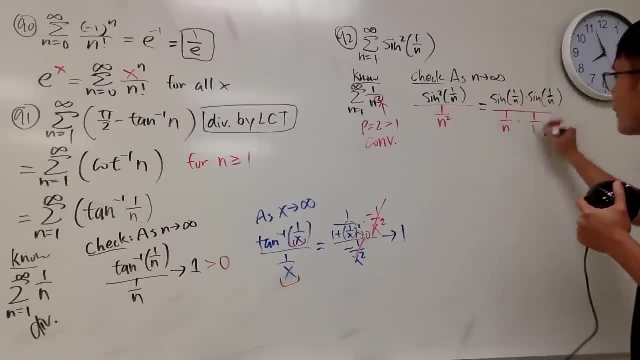 Sign Square Is The Same As A Sign Of One Over N Times. Sign Of One Over This Right Here Becomes Sign Of Theta Times. 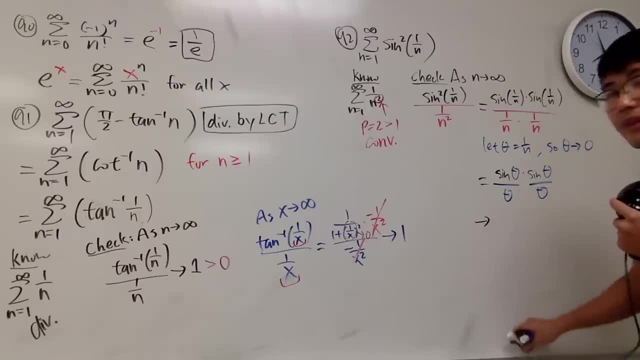 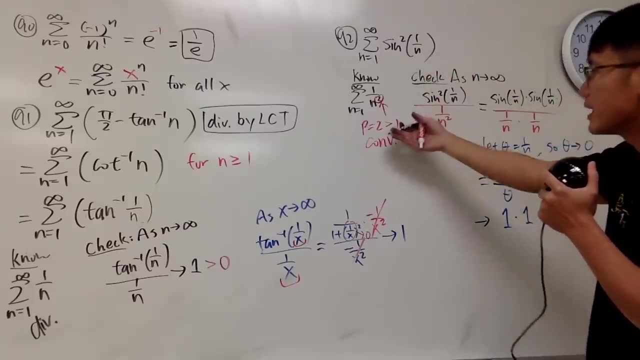 Sign Of Theta And We Have This, Divided By Theta, Divided By Theta, And This Right Here Approaches One And One You Just Use. 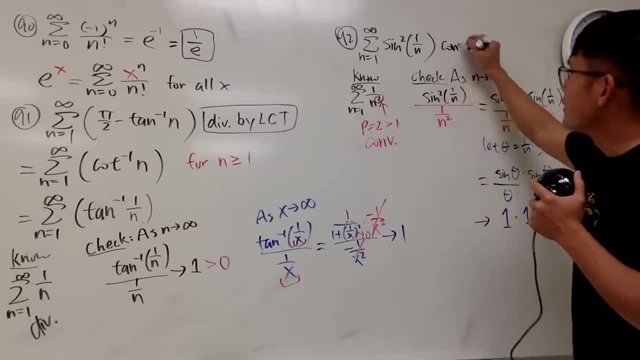 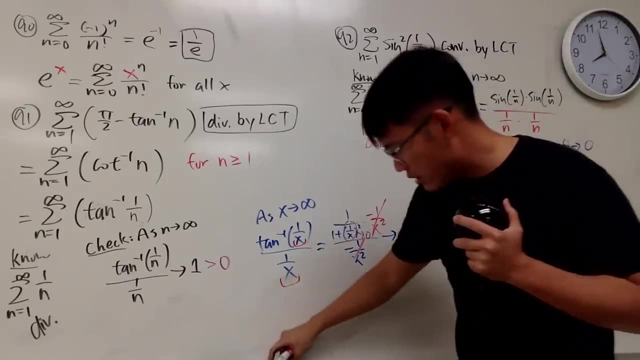 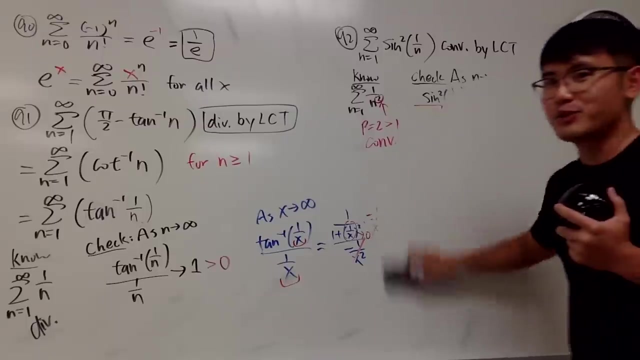 One Over N It's Not Good Right And This Right Here Also Converges. Why By The Limit Conversion Test L, C, T, L C. 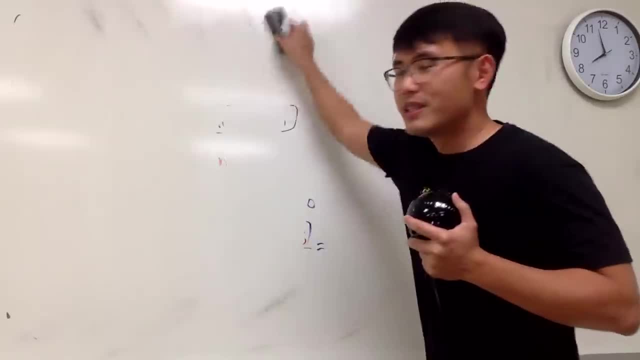 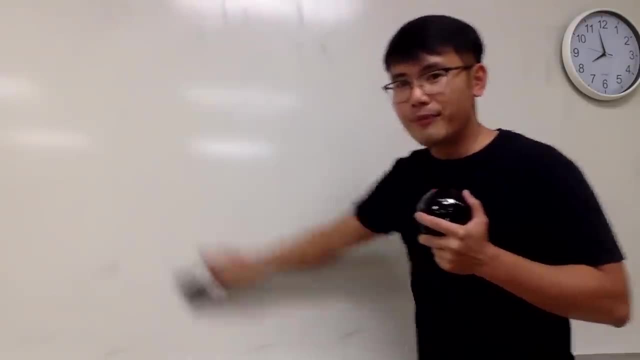 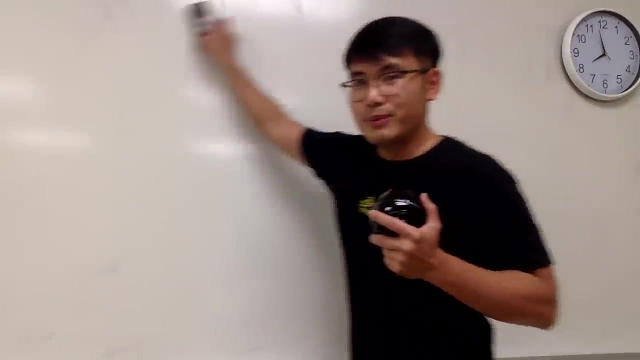 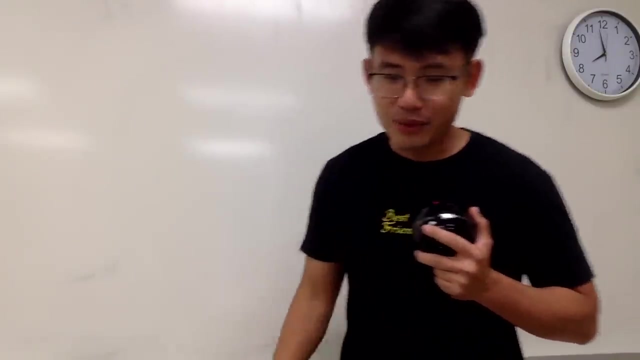 T L C P T T L Part This, So You To All The Students. Let Me Tell You, Of Course, The Best, Simple You Get. 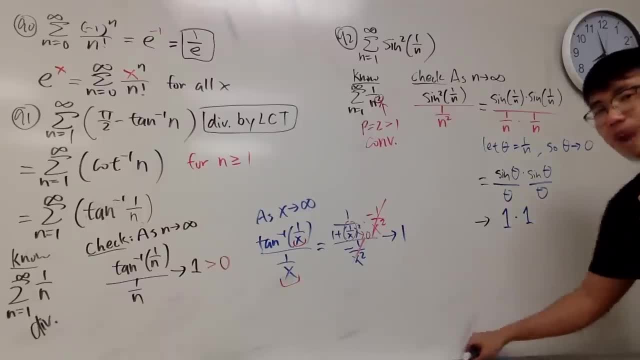 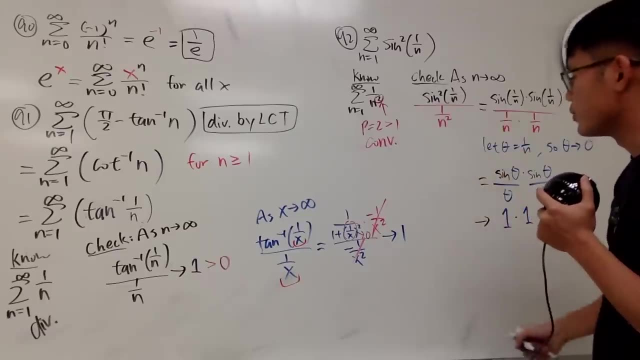 Of course, in the end this is just 1.. So again, this is also useful. This is greater than 0.. It's useful. Come back here, Draw the same conclusion, because this is greater than 0.. If you just use 1 over n, it's not good, right. 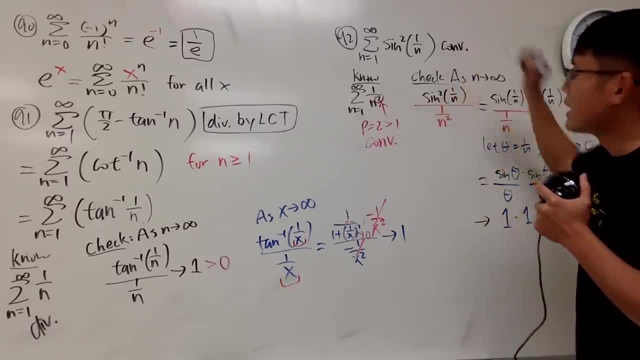 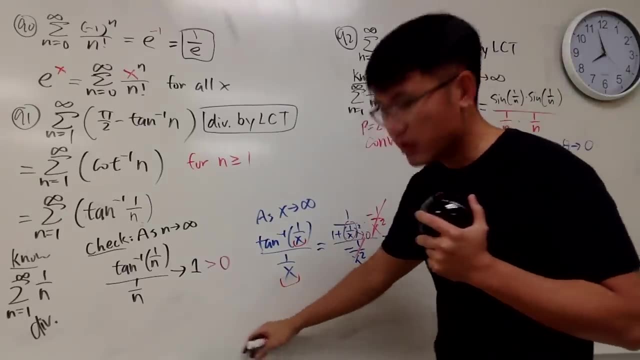 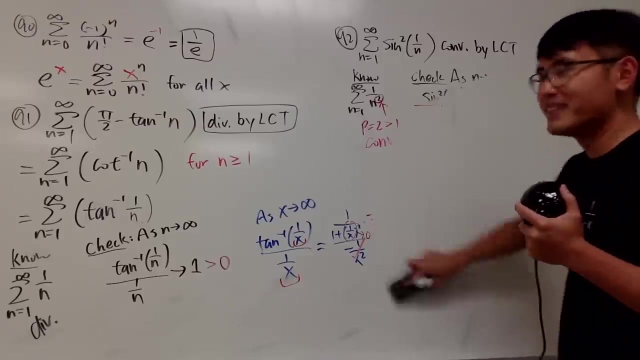 And this right here also converges. Why By the limit conversion test: LCT, LCT, LCT, right. So this right, here is it. Hopefully you guys also like, if not, just rewind it so you can like see what we did. 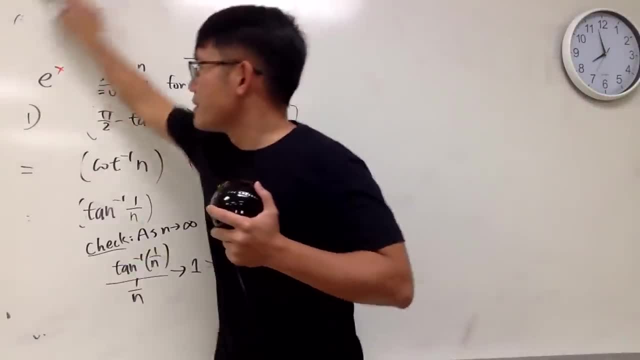 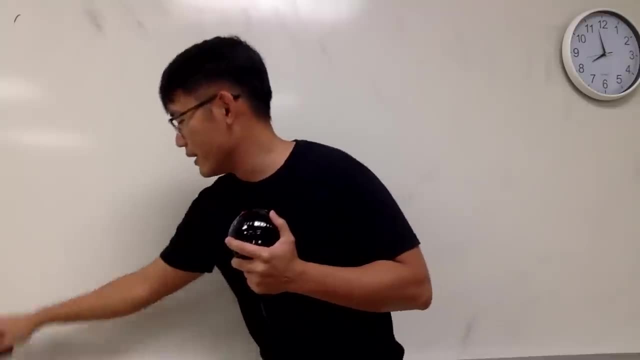 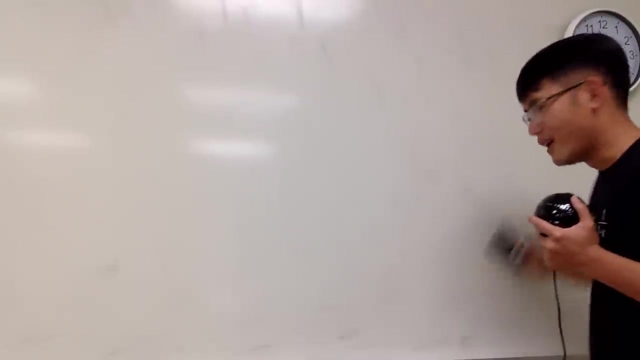 Okay, any more questions. Okay, any more questions. Okay, any more questions. You really feel this kind of excitement once you get to the last part, which is like you really have to work hard for these things. Yeah, So, to all the students, let me tell you, of course, 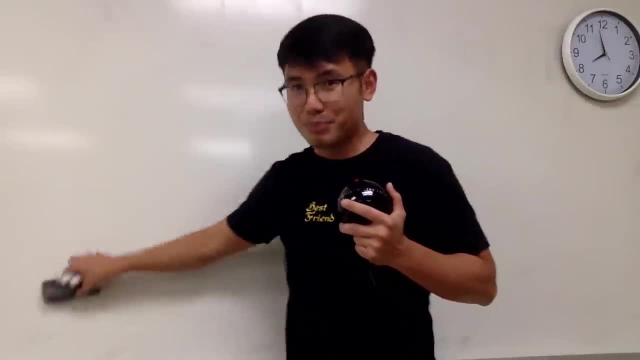 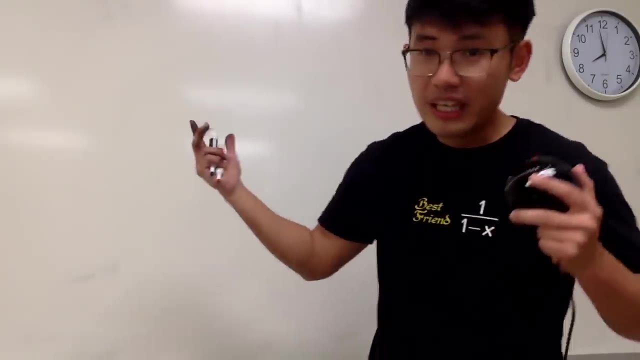 the best thing for you guys to do to get better is to practice, practice, practice. I won't tell you guys the things that I don't do. okay, I practice a lot myself too. If you don't believe it, this is the proof. 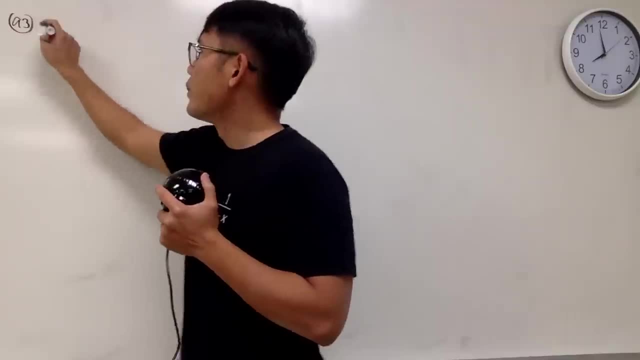 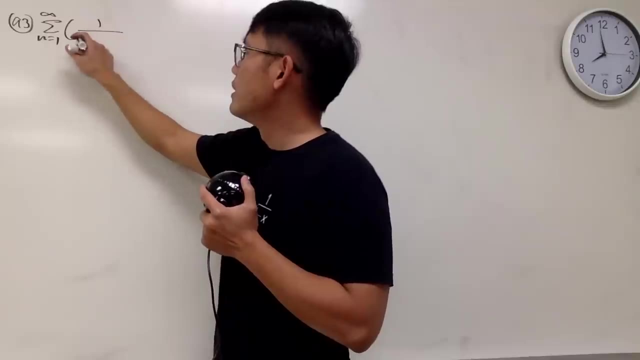 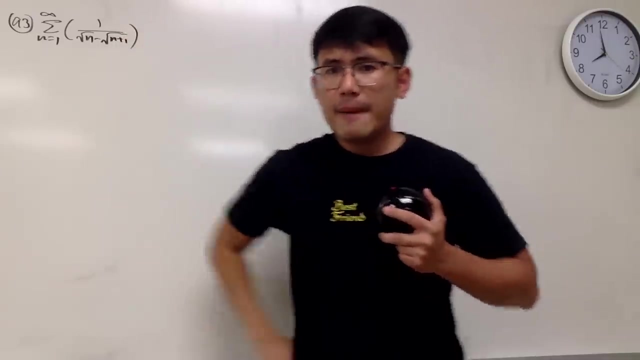 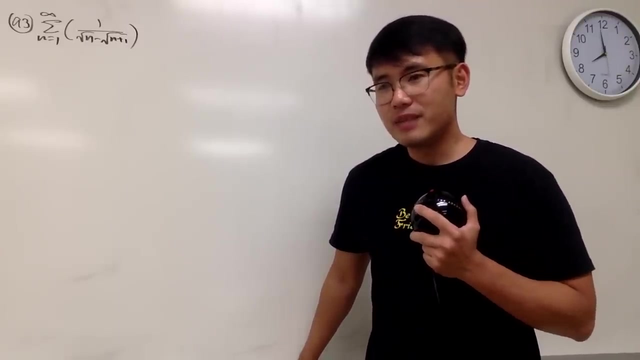 Anyway, Number 93.. Here we are going to look at the sum as n goes from 1 to infinity and we have 1 over square root of n minus square root of n plus 1.. Hmm, Hmm, Hmm, This right here is not telescoping. 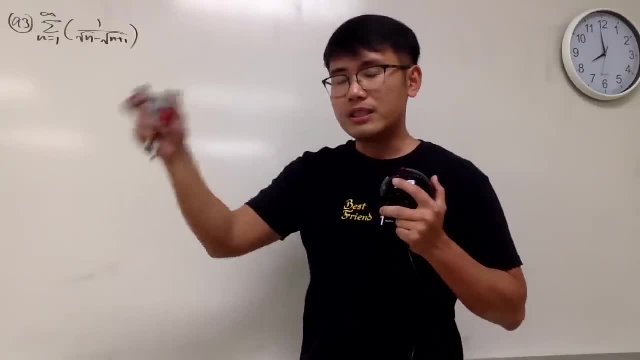 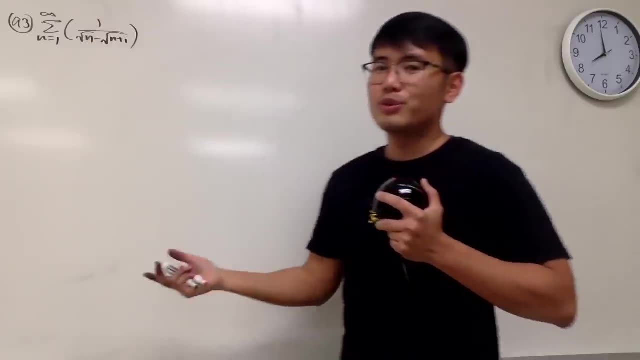 because it's not something minus the other, Like one turn. it's not bn minus, bn plus. Okay, you know, Inside here, in the denominator here, it's actually pretty bad. Okay, Let's see what can we do. 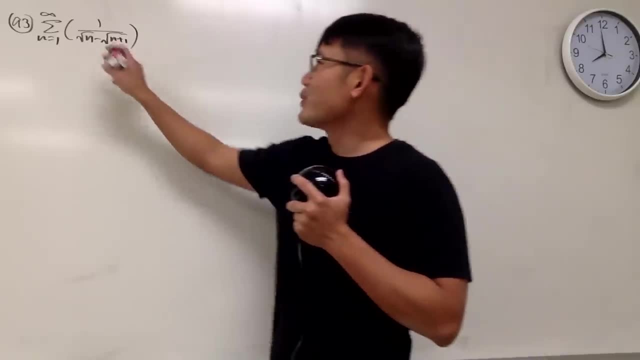 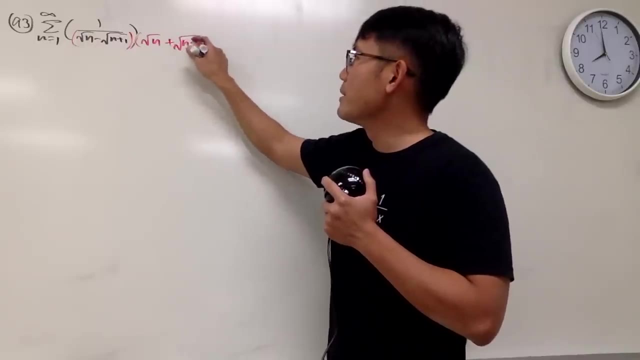 Let's take a look at the conjugate. How's that So? because whenever we have this right here, let's just go ahead and multiply the top and bottom by its conjugate, namely square root of n plus square root of n plus 1,. 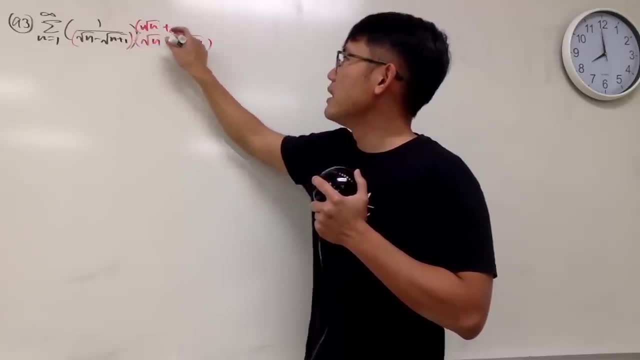 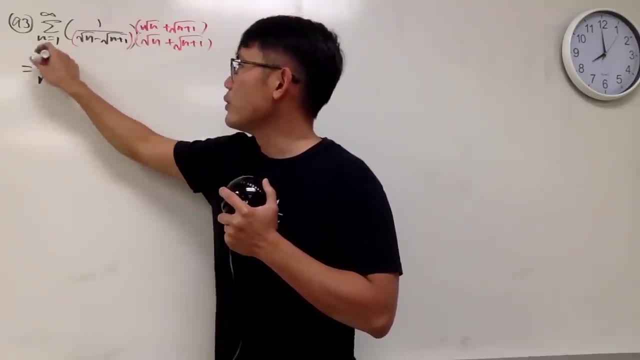 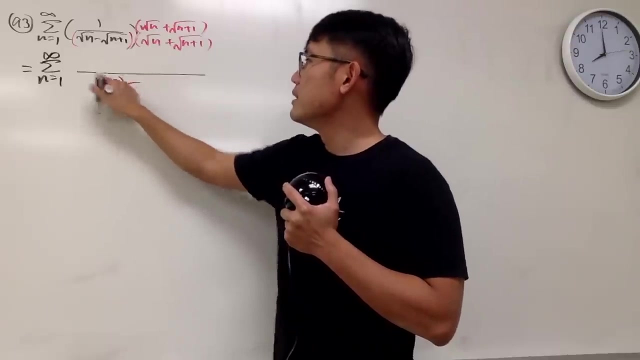 on the bottom and also on the top, And when we do that we see this is the sum, as n goes from 1 to infinity. And then for the denominator you have just n minus n plus 1.. Like that, And we'll just end up with a negative 1, right. 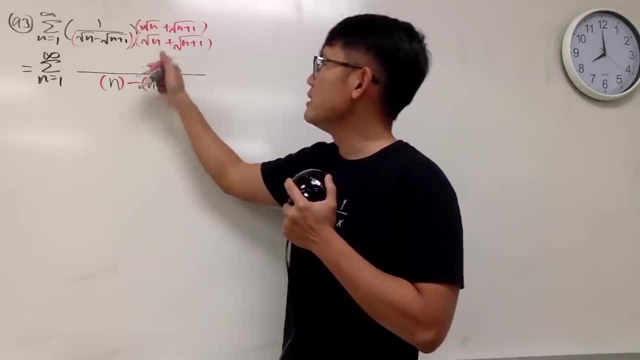 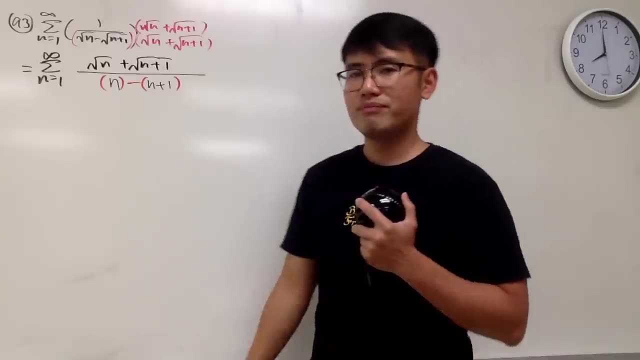 Well, if you look at this and that and you can see this is just square root of n plus square root of n plus 1. Like this. So, of course, if you want to do more, you can do a little bit more. 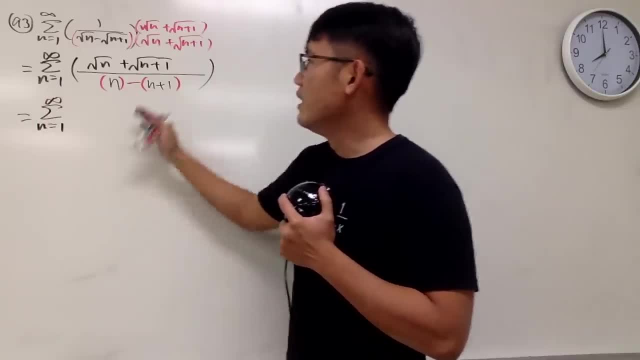 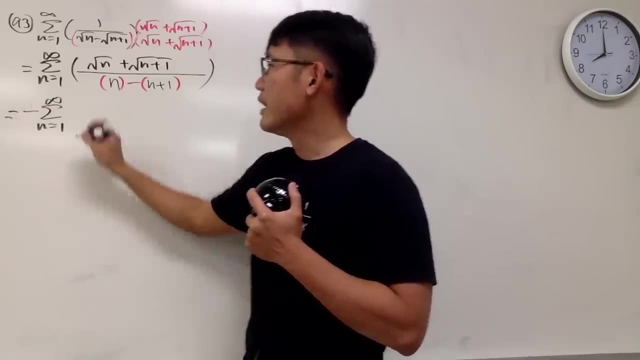 This is just the sum, As n goes from 1 to infinity, And this right here is just negative 1.. So, if you would like, you can actually take the negative all the way to the front And then you have square root of n plus square root of n plus 1.. 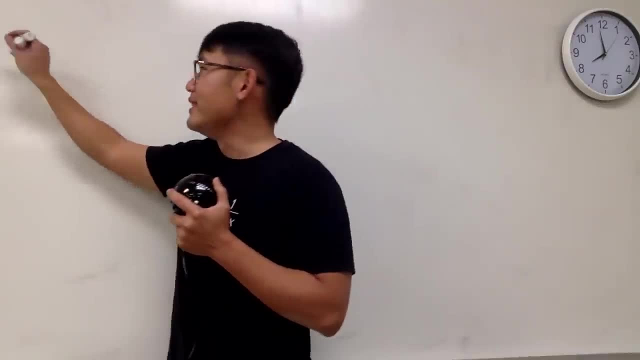 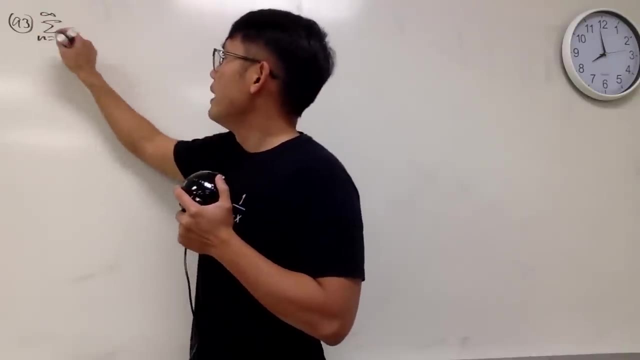 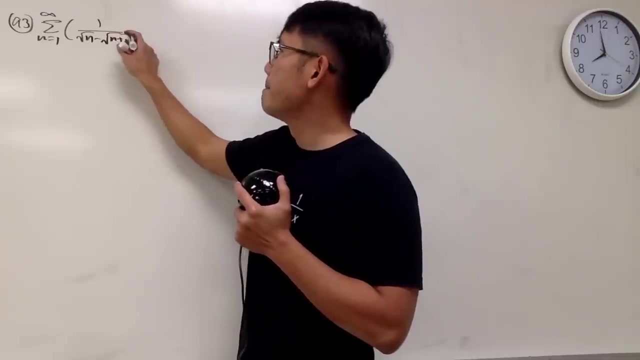 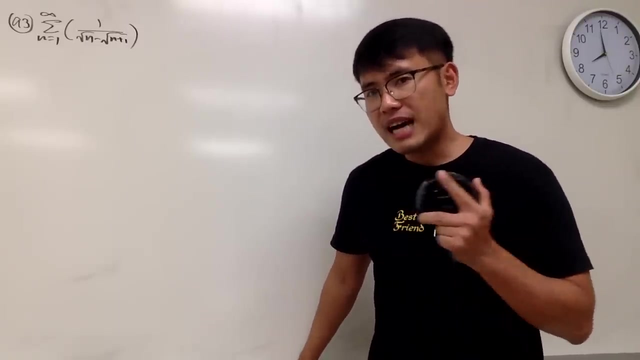 Better Is To Practice Practice. I look at the sum as n goes from 1 to infinity and we have 1 over square root of n minus square root of n plus 1.. This, right here, is not telescoping, because 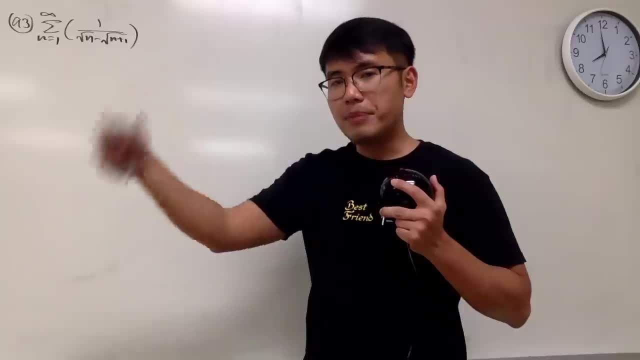 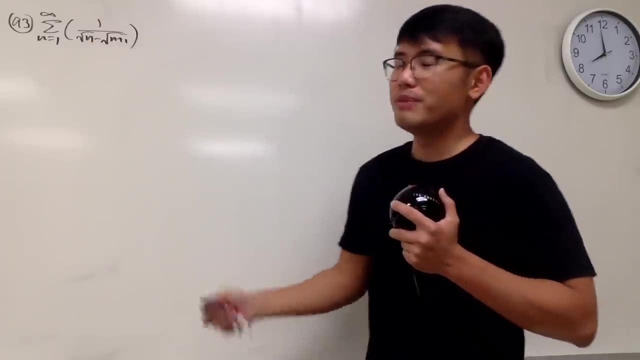 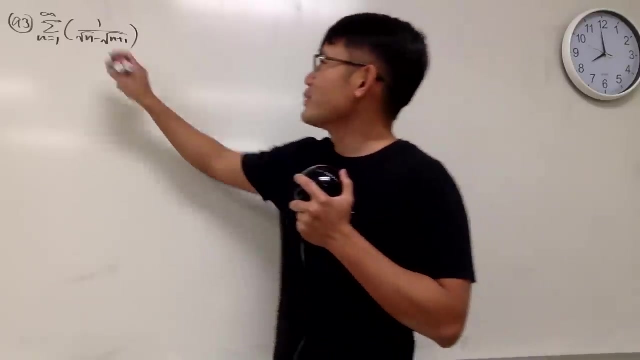 it's not something minus the other, like one term. it's not bn minus bn plus k Inside here, in the denominator here it's actually pretty bad. Okay, let's see what can we do. Let's take a look at the conjugate. how's that So? because whenever 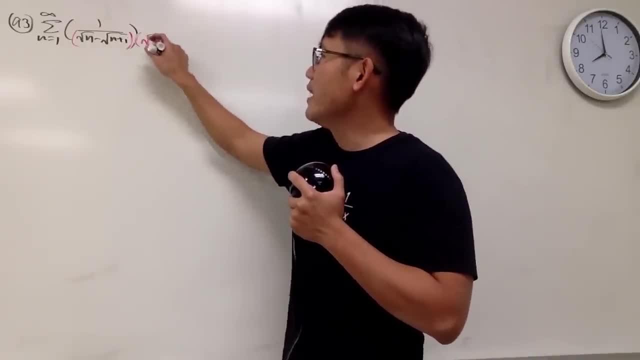 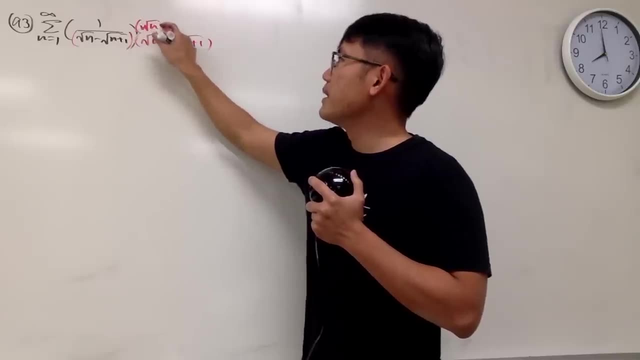 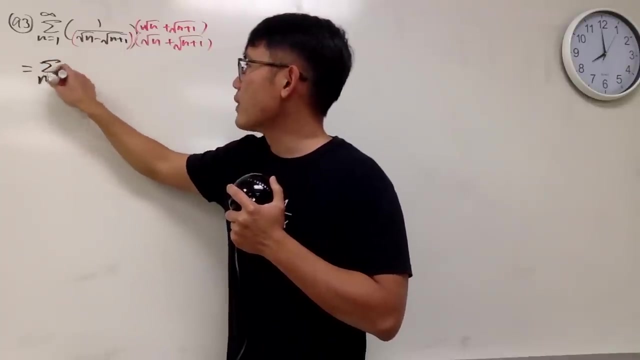 we have this right here. let's just go ahead and multiply the top and bottom by its conjugate, namely square root of n plus square root of n plus 1 on the bottom and also on the top, And when we do that, we see, this is the sum, as n goes. 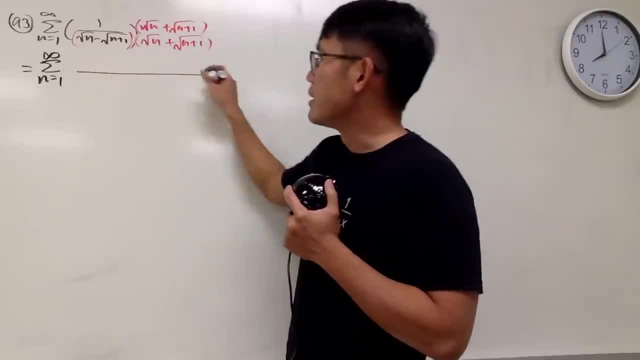 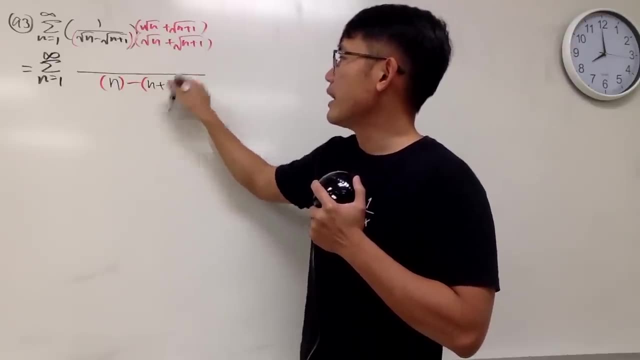 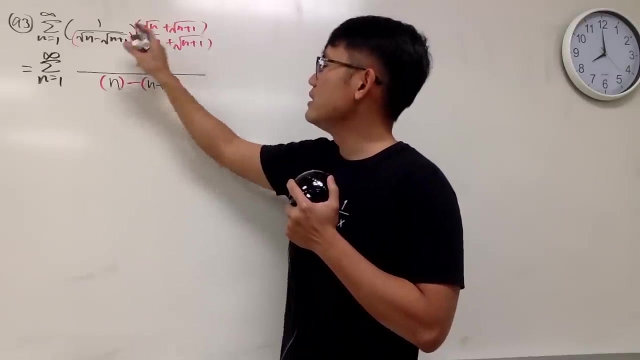 from 1 to infinity, And then for the denominator, you have just n minus n plus 1, like that, And we just end out with a negative 1, right? Well, if you look at this and that and you can see this, 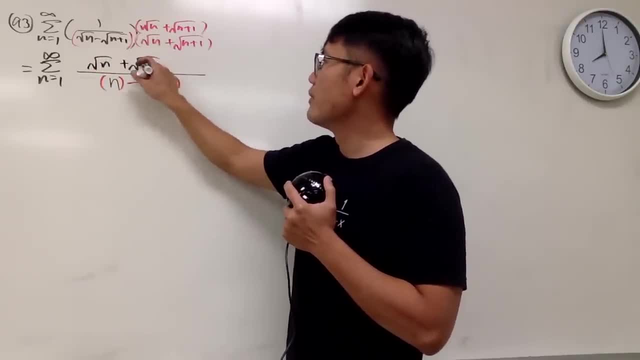 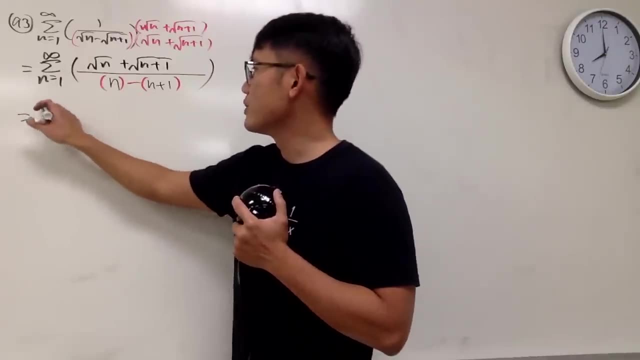 is just square root of n plus square root of n plus 1, like this. So, of course, if you want to do more, you can do a little bit more. This is just the sum, as n goes from 1 to infinity. 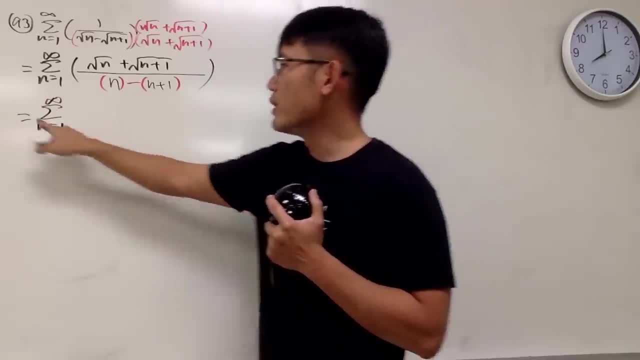 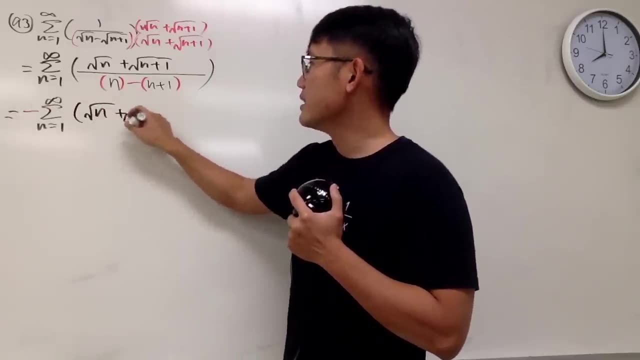 and this right here is just negative 1.. So, if you would like, you can actually take the negative all the way to the front and then you have square root of n plus square root of n plus 1.. But you guys know this, as n goes to infinity. this right here. 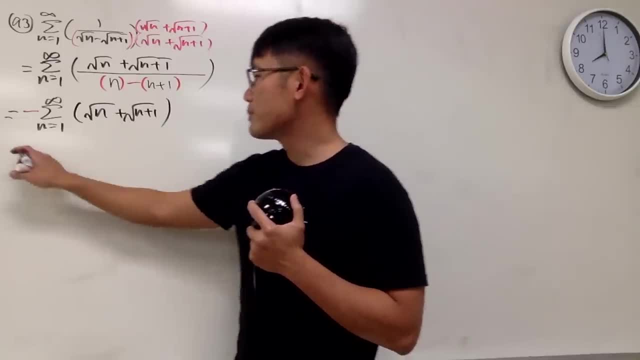 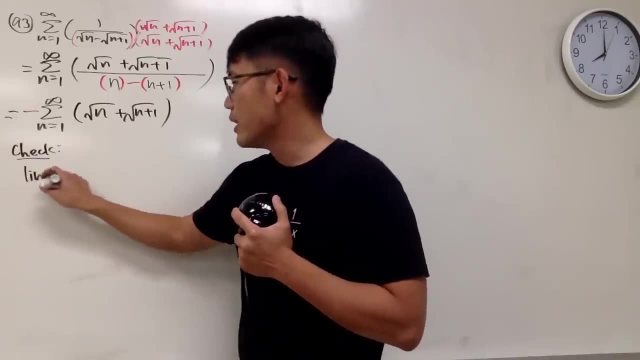 actually goes to infinity right. So I will just put this down here real quick for you guys. So test for divergence. we check. let's just write this down real quick: The limit as n goes to infinity of 0, you can put, you can include a negative right here as well, if you would like. I think 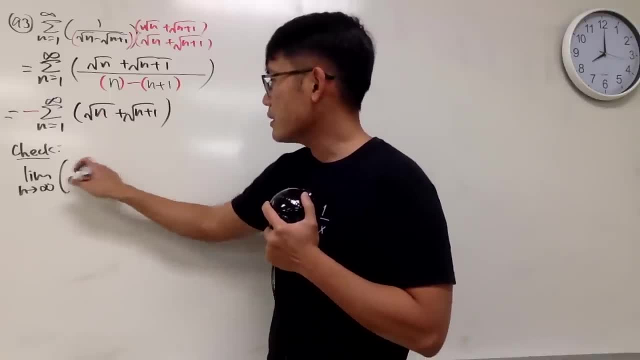 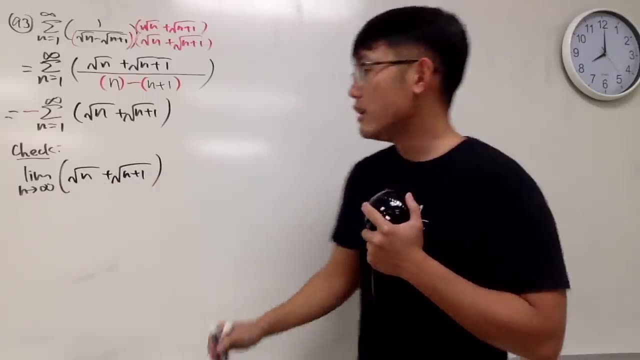 oh. however, you guys should know, the negative is in front. So this right here, square root of n plus square root of n plus 1, this is just adding infinity plus infinity. that has to be infinity. Therefore, this right here is equal to infinity, which is not 0, done This right here. 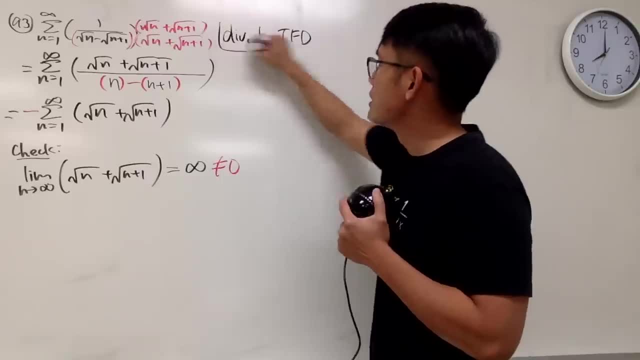 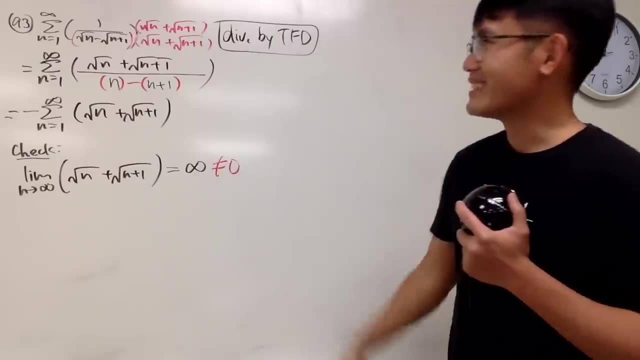 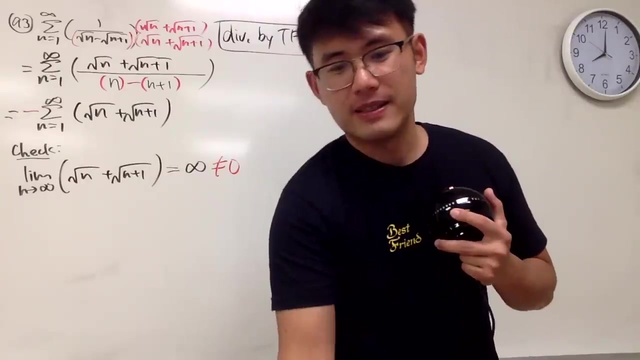 divergence by test for divergence. If I'm to take the limit right away, you will have to multiply by the conjugate anyway. So that's the idea, right here, right? So that's it. Now guess what We're done with this? 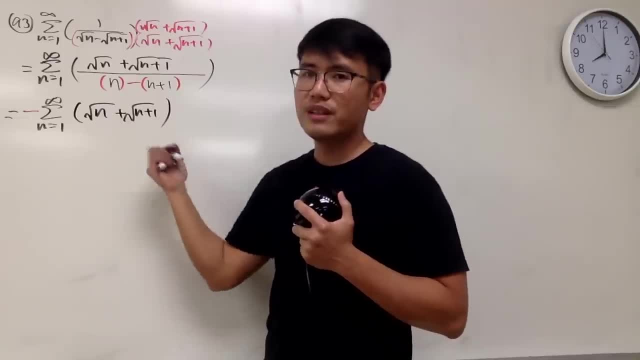 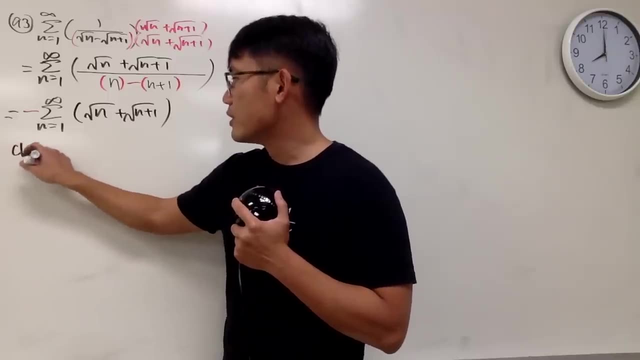 But you guys know this, As n goes to infinity, this right here actually goes to infinity, Right. So I will just put this down right here real quick for you guys. So test for divergence, We check. Let's just write this down real quick. 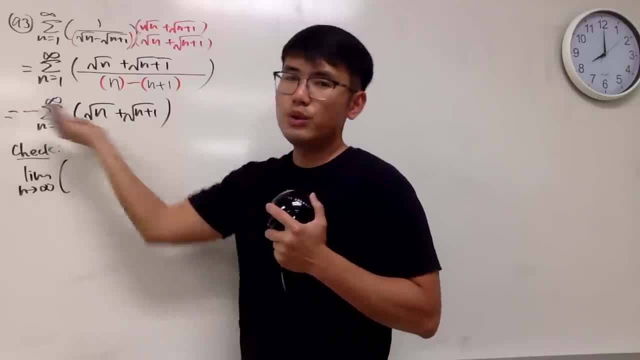 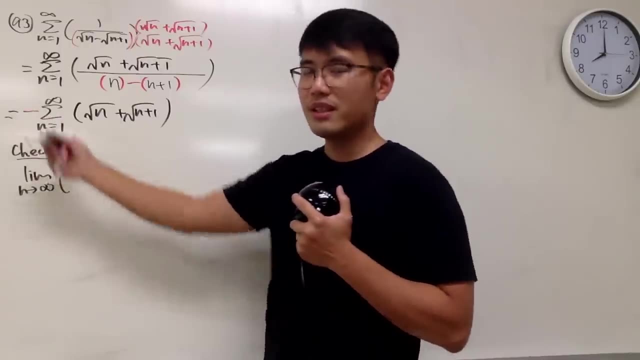 The limit, Okay, As n goes to infinity- of You can put. You can include negative right here as well, if you would like. I think, However, you guys should know the negative is in the front. So this right here: square root of n plus square root of n plus 1.. 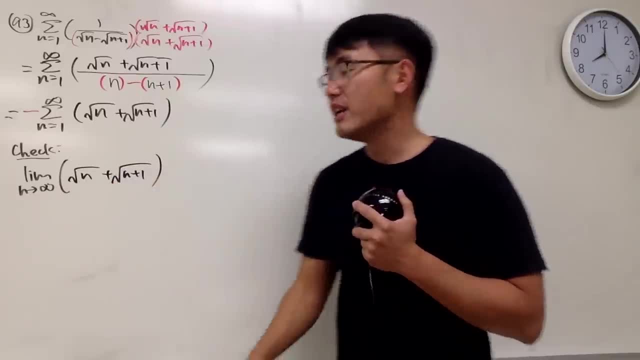 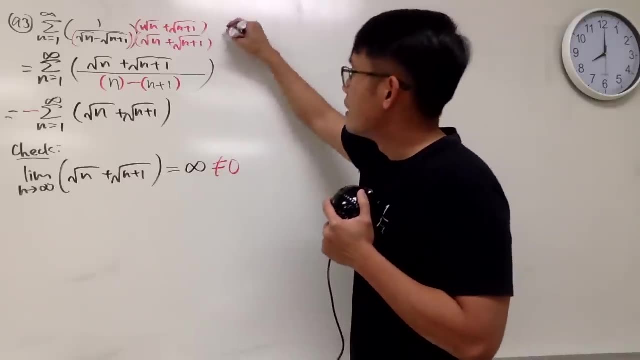 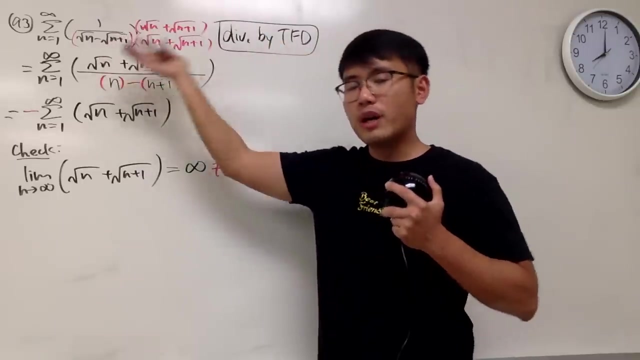 This is just adding infinity plus infinity. That has to be infinity. Therefore, this right here is equal to infinity, which is not 0. Done, This right here diverges by test for Divergence And if you want to take the limit right away. 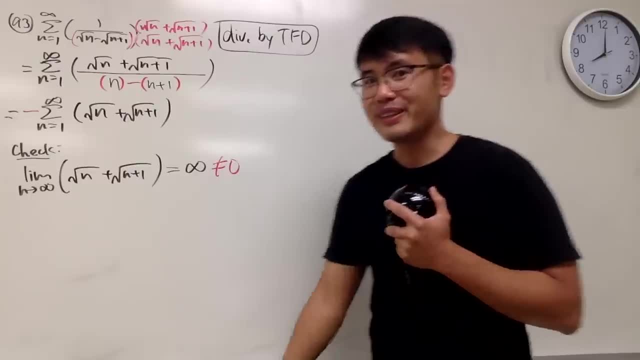 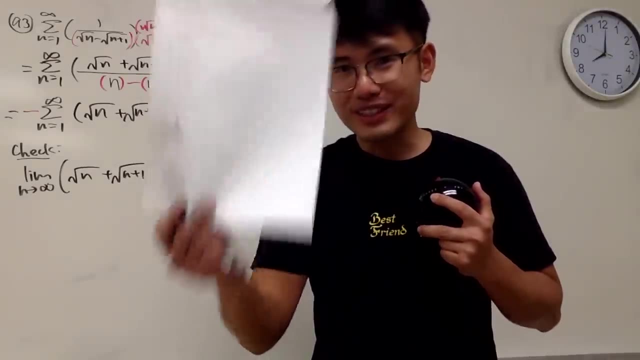 you will have to multiply it by the conjugate anyway. So that's the idea, right here. Right, So that's it. Now Guess what We're done with this. So good, Last page, Last page, Last page. 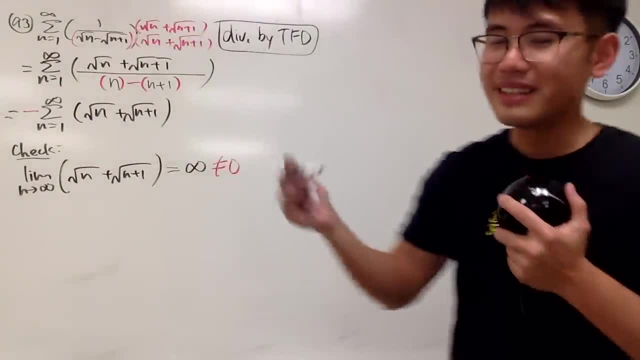 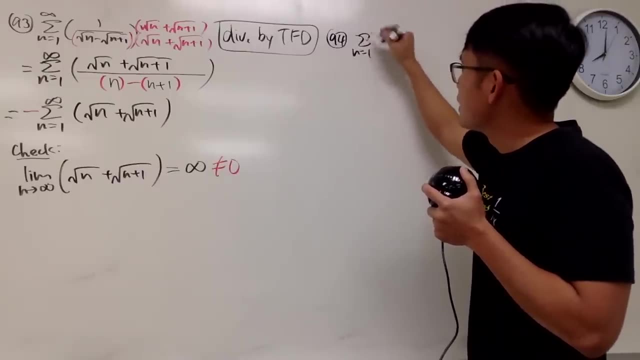 This one, we have 1 over square root of n. Oh man, Telescoping finally. huh, So 94.. Let's get going. Okay. N goes from 1 to infinity, 1 over square root of n minus 1 over square root of n plus 1.. 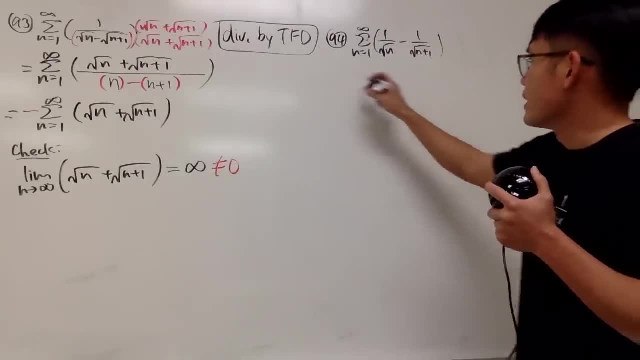 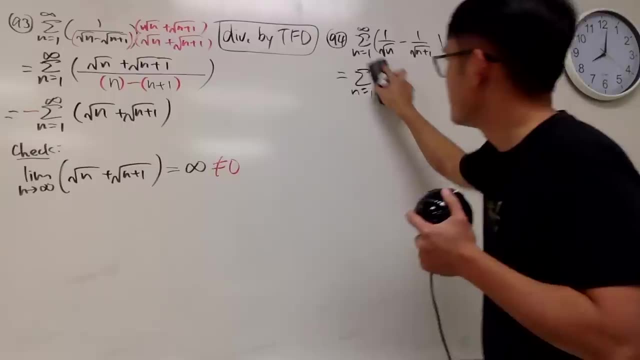 Like that Right Geome Telescoping. So let's go ahead and just telescope this guy. And I'll just show you guys: n is equal to 1.. Well, actually that will expand that. So when you put in 1, you get 1 over square root of 1 minus 1 over square root of 2.. 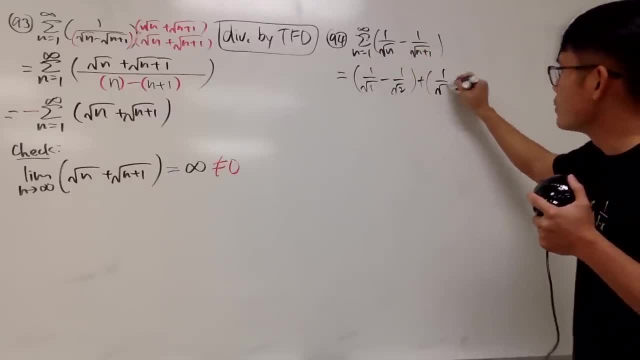 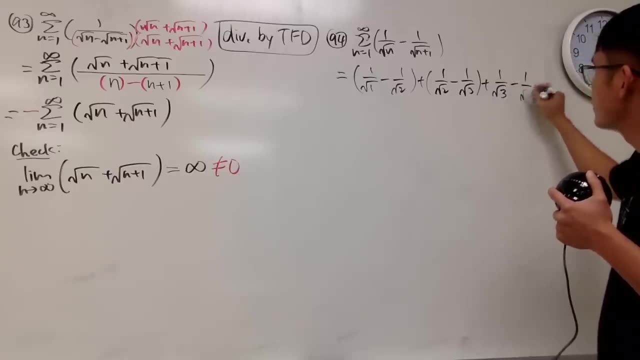 And then you add The next time you put in 2. So you get 1 over square root of 2 minus 1 over square root of 3.. And then plus 1 over square root of 3 minus 1 over square root of 4.. 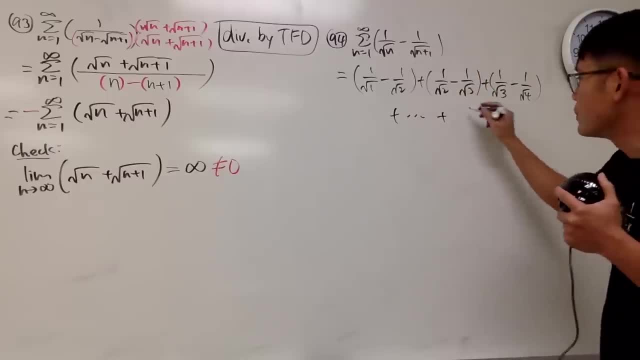 And then plus, Da, da da, Plus the n-th term. You also put this down, Which is 1 over square root of n minus 1 over square root of n plus 1.. Plus, da, da da. 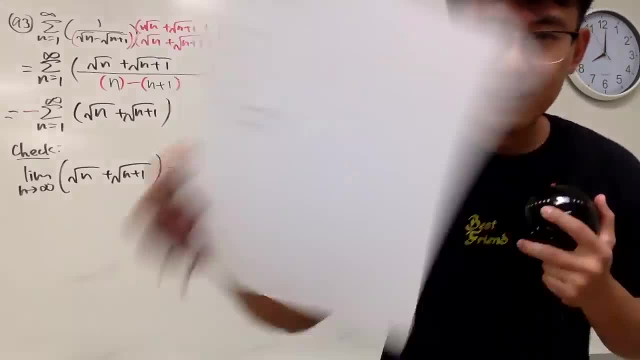 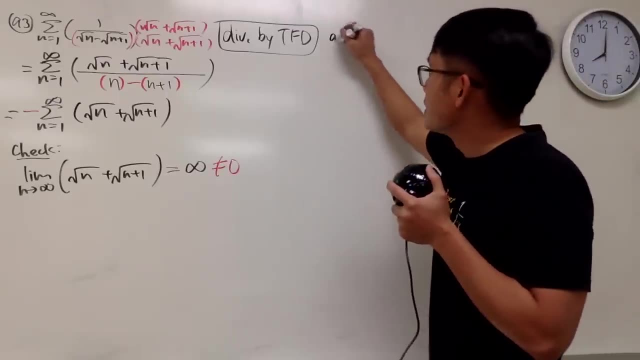 So good, last page, last page, last page, This one- we have 1 over square root of n. Oh man, geomagnetism, uh, telescoping, finally, huh, So 94, let's get going. N goes from 1 to infinity, 1 over square root of n plus infinity. 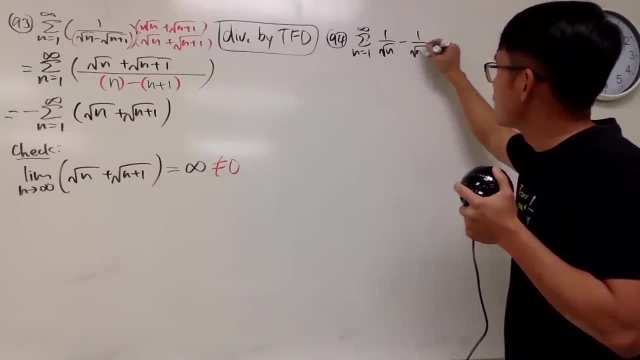 So that's it right. So here's Germany's increment to infinity from infinity 1 over on finishes. So we are done right. so this is one comum we can write. so this is a square root of n minus 1 over square root of n plus 1, like that right geom telescoping. so let's. 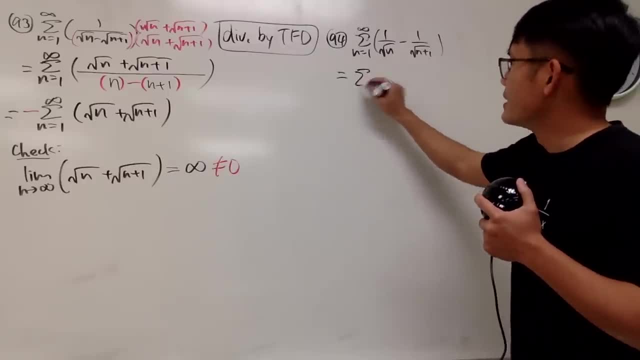 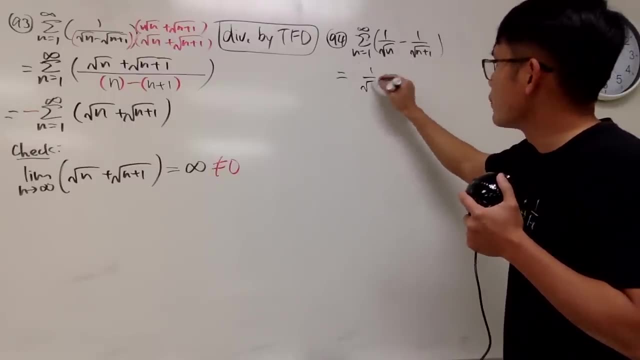 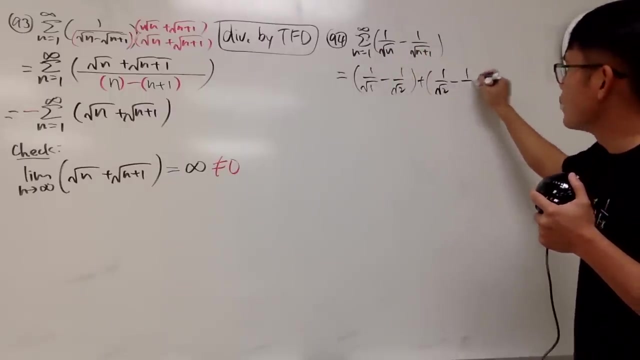 go ahead and just telescope this guy and i'll just show you guys, n is equal to 1. well, actually that will expand that. so when you put in 1, you get 1 over square root of 1, minus 1 over square root of 2, and then you add the next term, you put in 2, so you get 1 over square root of 2 minus 1 over. 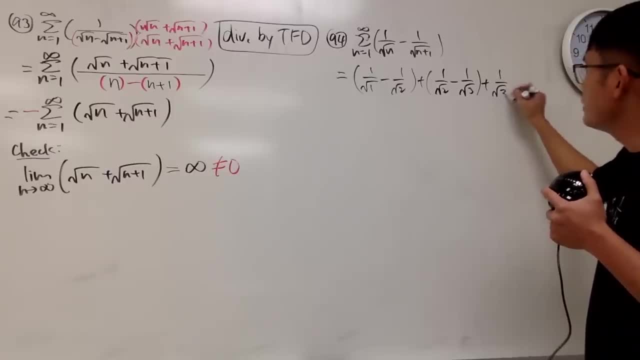 square root of 3, and then plus 1 over square root of 3, minus 1 over square root of 4, and then plus plus the nth term. you also put this down, which is 1 over square root of n, minus 1 over square root. 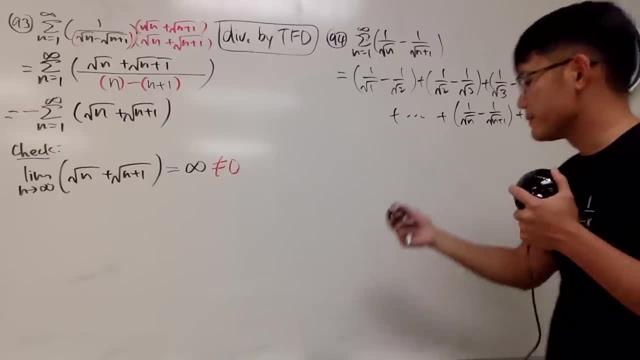 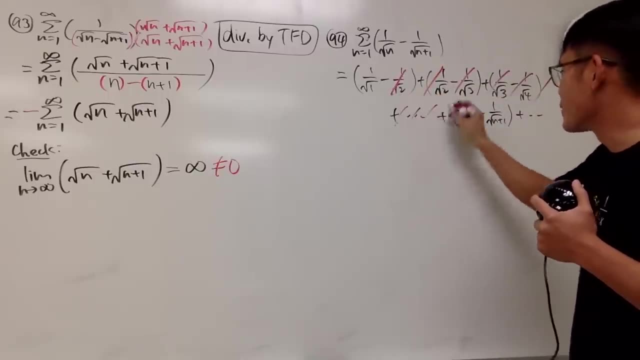 of n plus 1. plus you know the deal: this guy and that guy cancel. this guy and that guy cancel this guy and something else. next guy will cancel, cancel, cancel, cancel, cancel. this guy and this guy will also cancel. you have this being 1 and then you have 1 minus square root of n plus 1, notice this. and that is just off by 1. 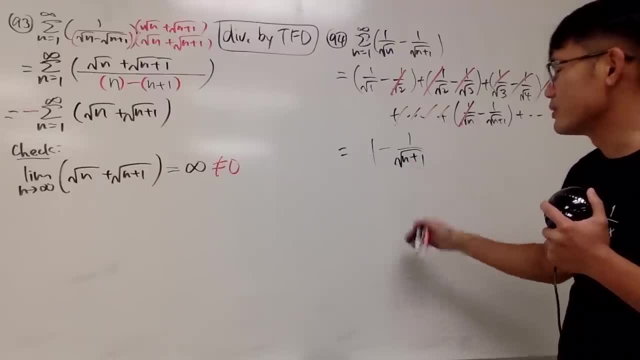 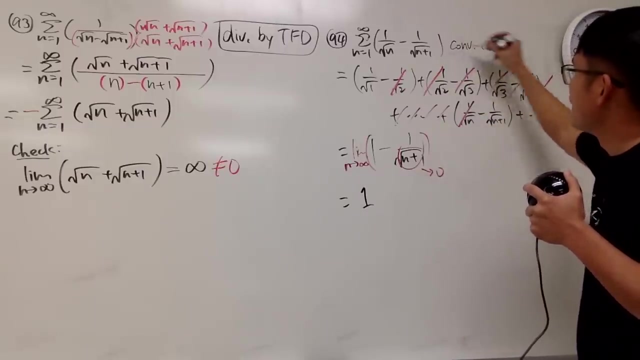 right n and n plus 1, just off by 1, even though they have the square root. but one term, one term. take the limit now, as n goes to infinity. you know, this right here is 1, because this right here goes to 0, so converges to 1, telescoping. 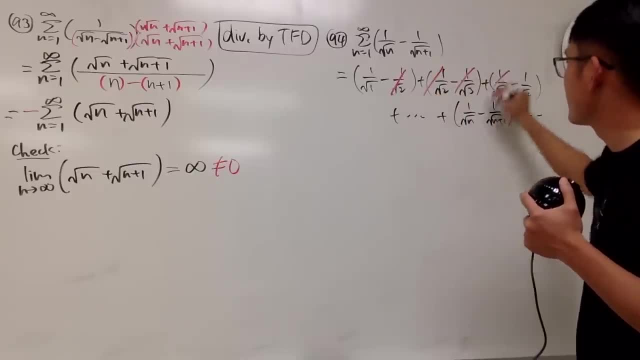 You know the deal: This guy and that guy cancel, This guy and that guy cancel, This guy and something else. Next guy will cancel, Cancel, cancel, cancel, cancel. This guy and this guy will also cancel. So you have this being 1.. 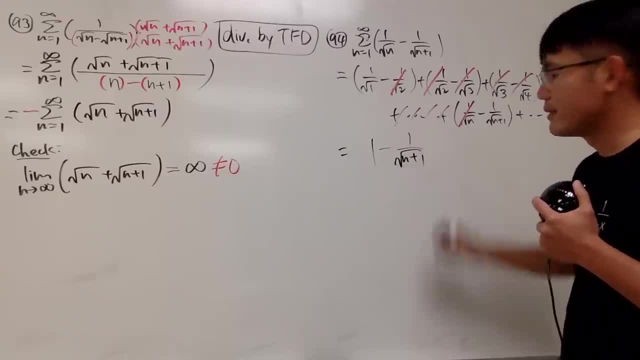 And then you have 1 minus square root of n plus 1.. Notice this. and that is just off by 1.. Right n and n plus 1 is just off by 1. Even though they have the square root. 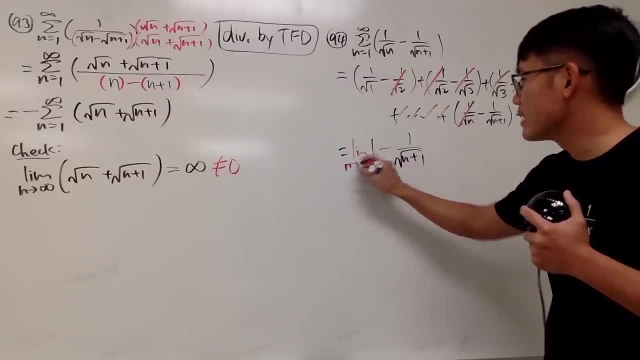 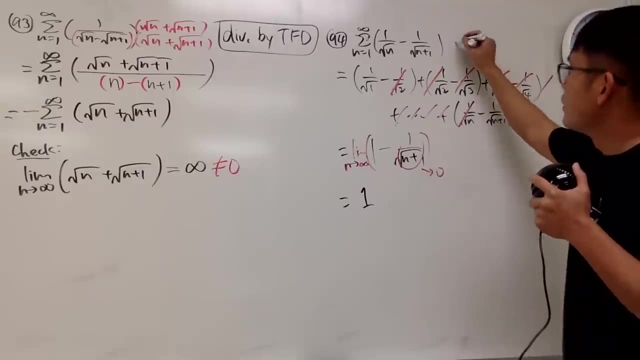 But one term, one term. Take the limit now, As n goes to infinity. You know this right here is 1.. Because this right here goes to 0. So converges to 1.. Telescoping Right. 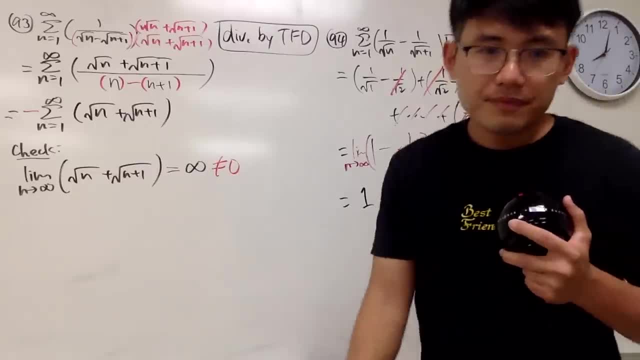 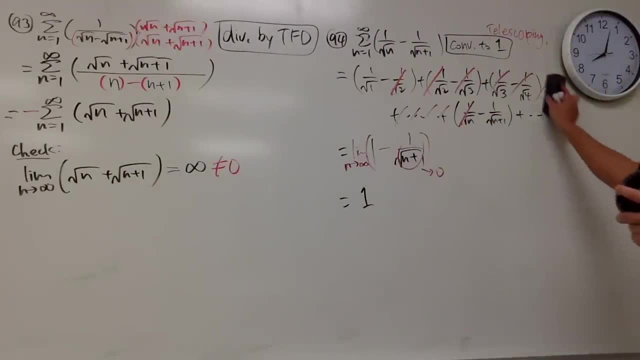 So That's the idea. Okay, I should put that as one of the hundred questions we saw, But like No, no, no, no, no, no, No worry. So for this one, if you do any kind of computers. 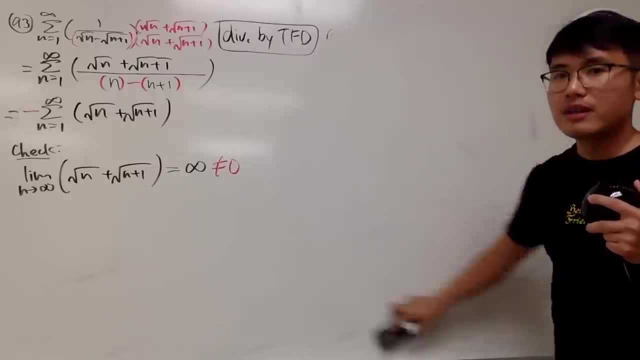 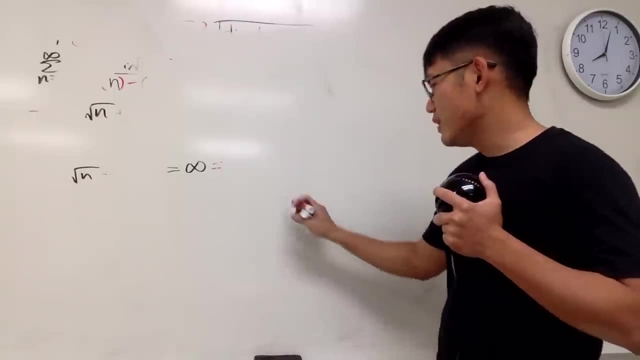 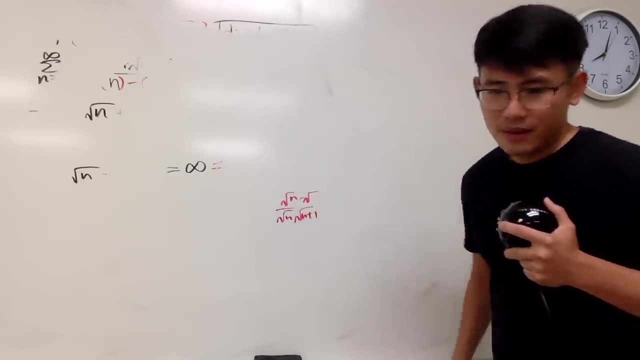 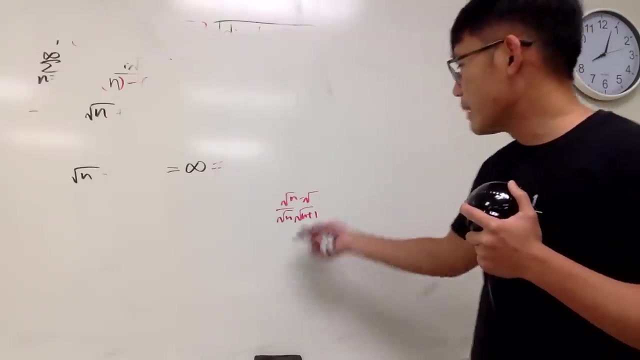 then you can also do so. You can also get a common denominator and then just work things out. I think that will work. Does it Wait? Did you get a common denominator? Huh, Hold on. Uh, Oh, yeah, you get a common denominator. 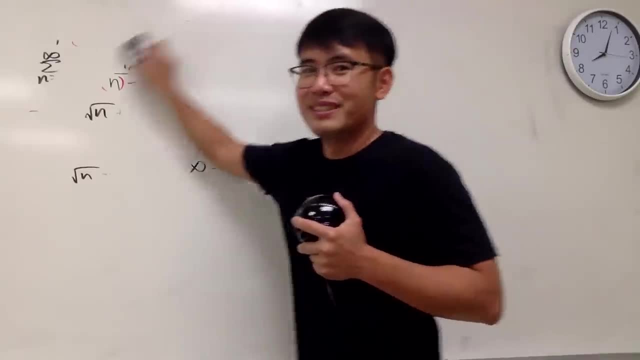 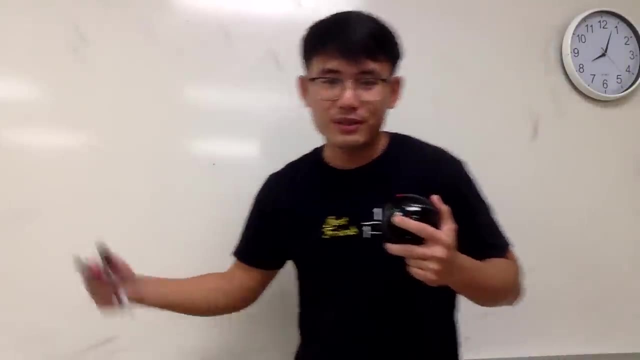 and then you do the conjugate. So yeah, It still works. It still works, I think, so Just do it on your own, But I solved it for you guys, So no complaining. e to the square root of n. 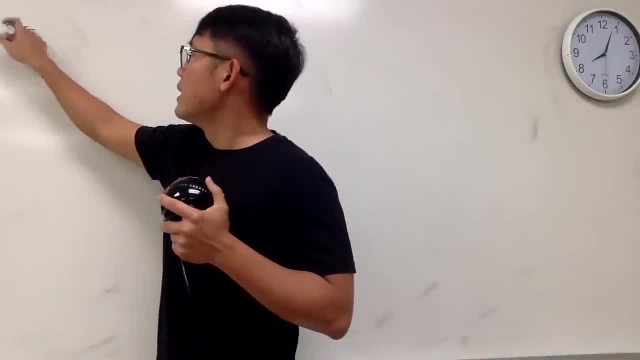 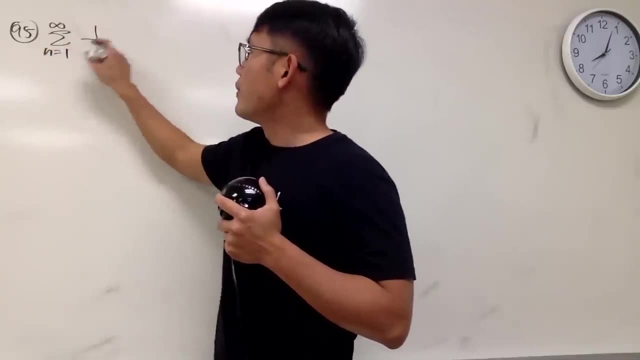 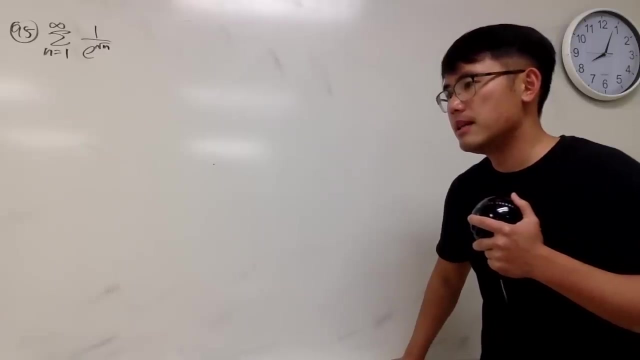 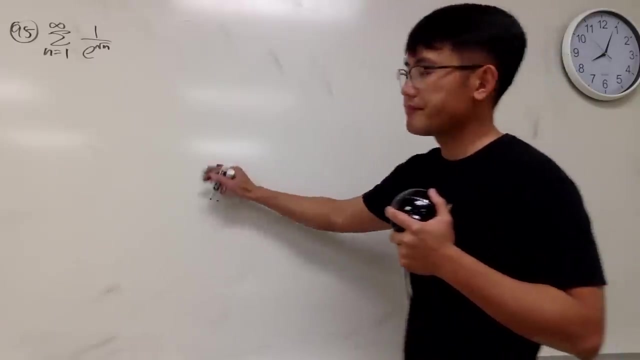 Oh my god, Number 95.. Sum As n goes from 1 to infinity, 1 over e to the square root of n. Hmm, I think this right here converges. I'm going to prove it by claim that I know. 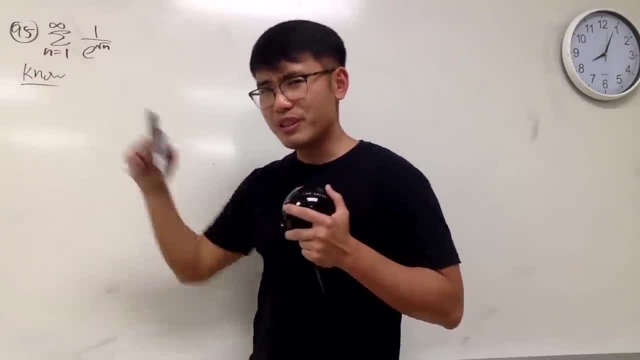 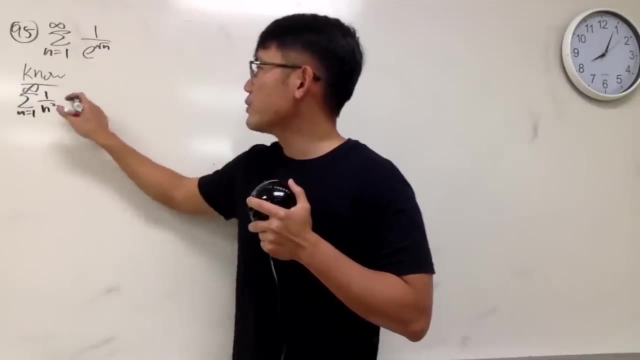 1 over n squared converges. We'll just make a quick comparison right. So the sum as n goes from 1 to infinity. this right here converges Why? I don't know how many times we've done it. 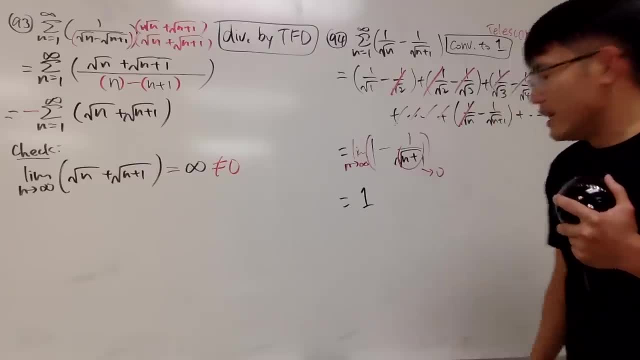 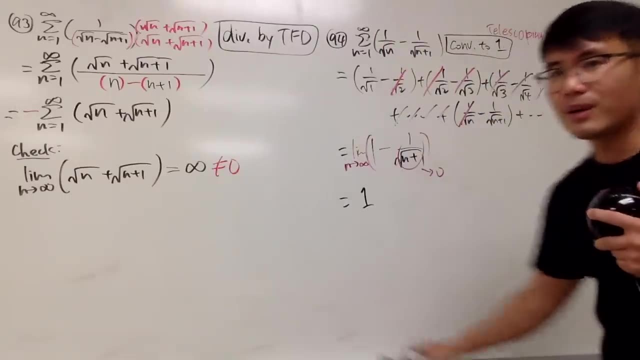 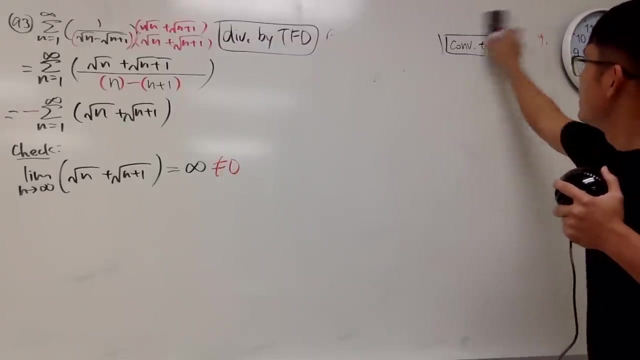 right, so that's the idea. okay, i should put that as one of the 100 questions or so. but like, uh, no, no, no, no, no, no worry. so for this one, if you do any kind of computation, you can also do so you can also get a common denominator and then just work things out. i think that will work. 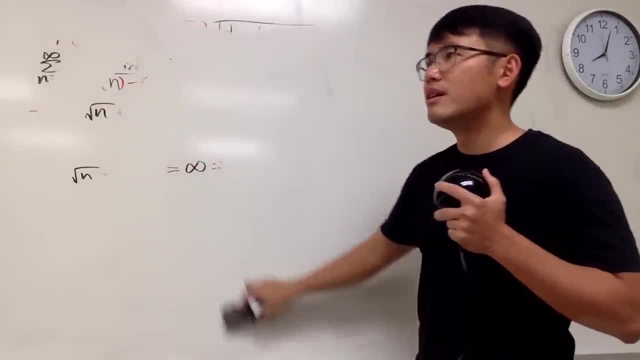 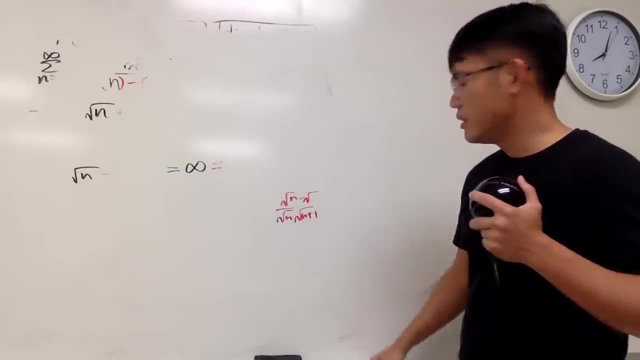 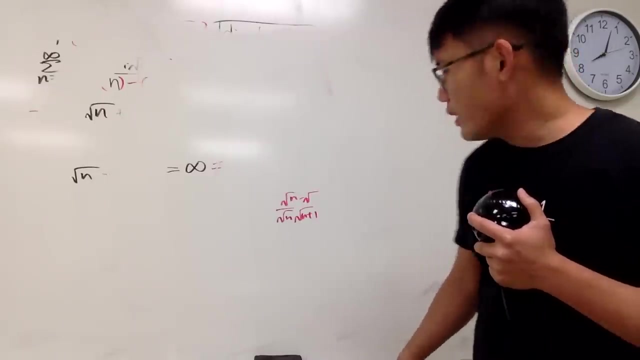 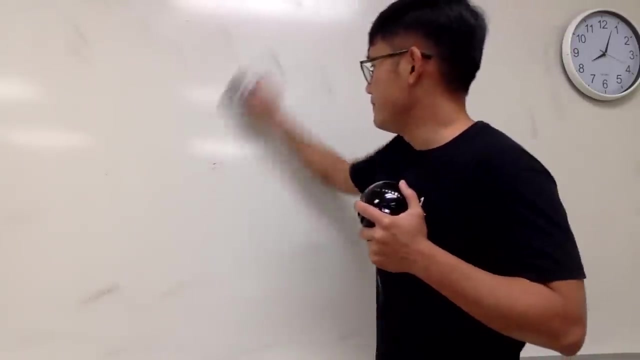 does it wait if you get a common denominator- huh, hold on, uh, oh yeah, good common denominator, and then you do the conjugate. so yeah, it's just, it'll still work. it still work, i think. so, like, just just just do on your own, but i solved it for you guys. so 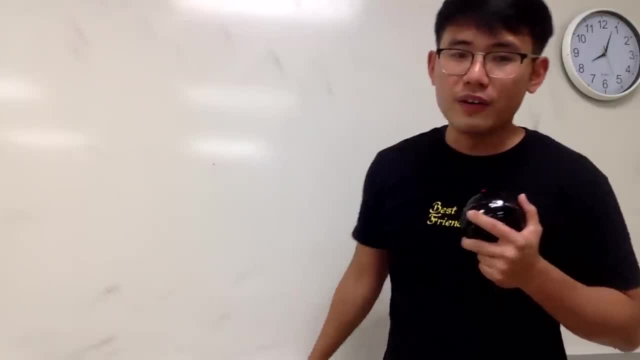 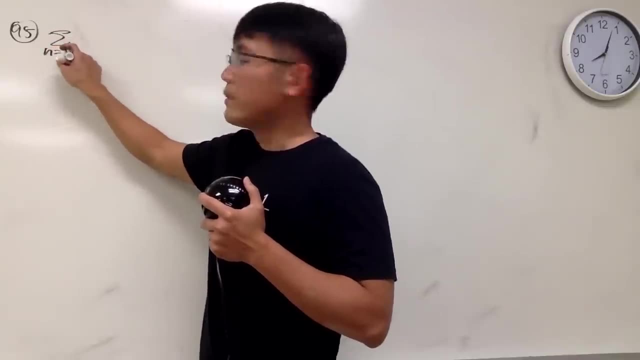 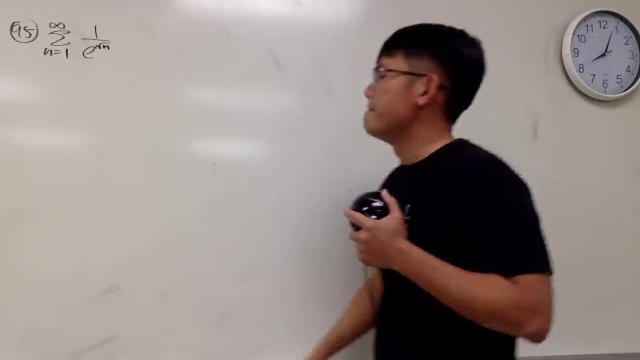 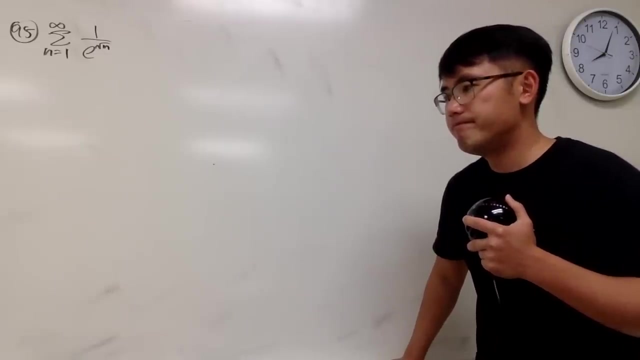 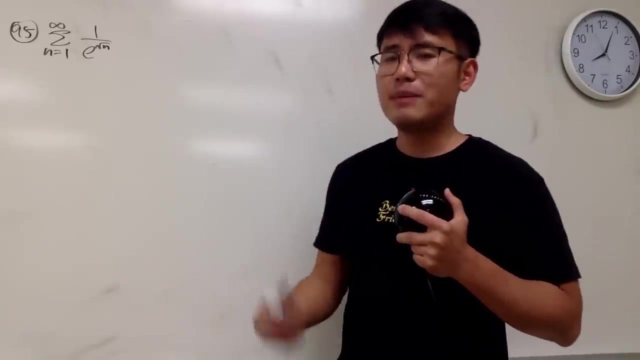 no complaint. right e to the square root of n. oh my god, number 95. uh sorry, as n goes from 1 to infinity. 1 over e to the square root of n. Hmm, I think this, right here, converges. I'm going to prove it by claim that I know 1 over n squared converges. 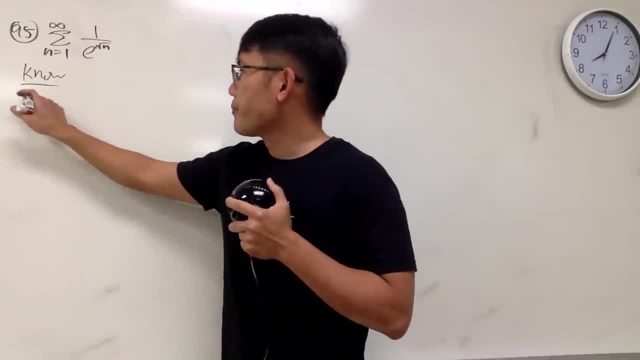 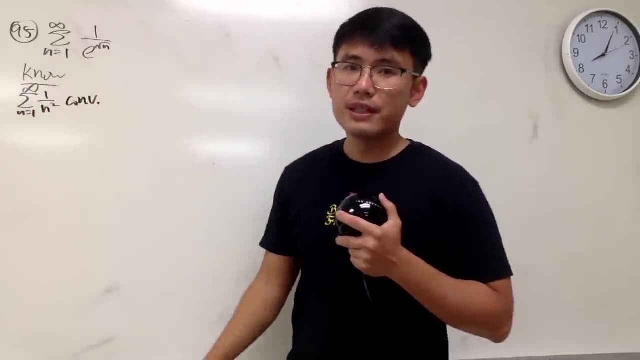 We'll just make a quick comparison, alright. So the sum as n goes from 1 to infinity. this right here converges Why. I don't know how many times we've done it, but just write it down seriously. 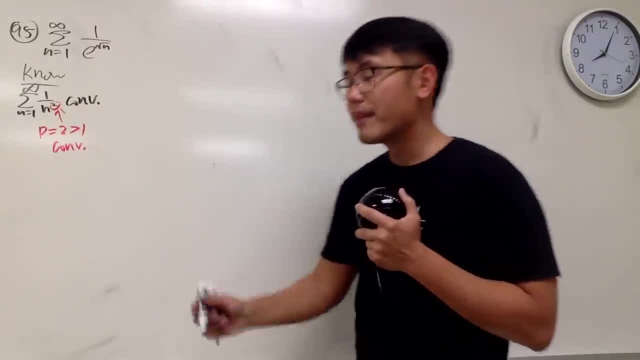 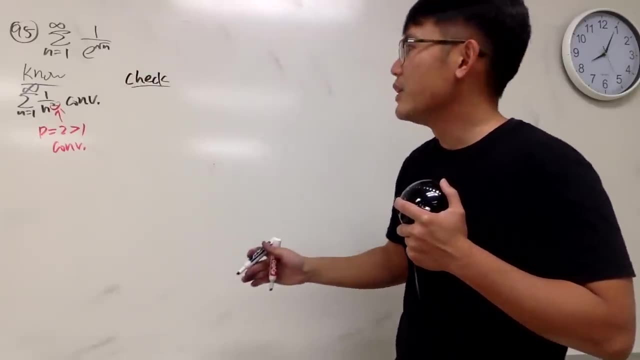 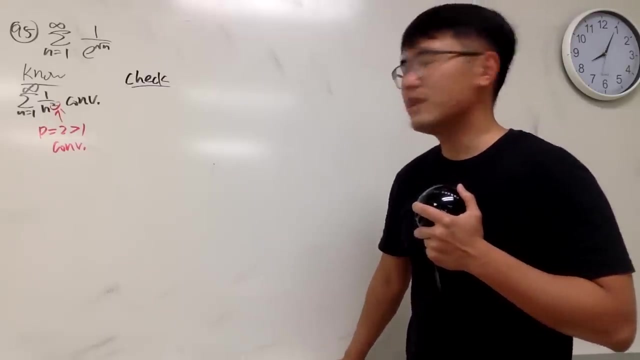 Converges P-series. Thank God, Now we will do a real quick comparison. so this is just going to be a direct comparison. You will see You can also do a. You can also do a limit. Why didn't I do a limit earlier? 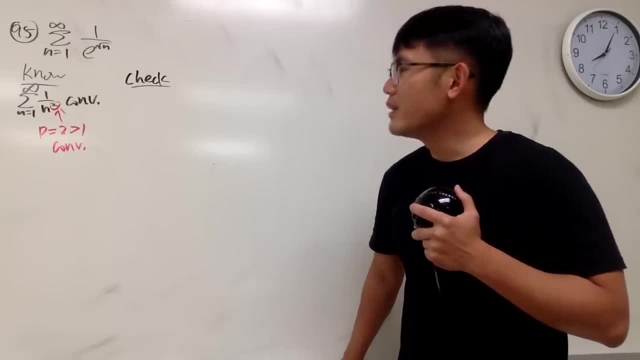 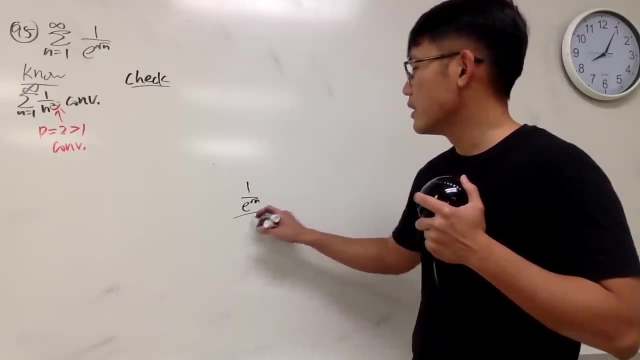 Yeah, why didn't I do a limit earlier? If I do a limit comparison, Let me see 1 over e to the square root of n. Oh yeah, it's not going to be a nice value. I have to take this as a special case for that also. 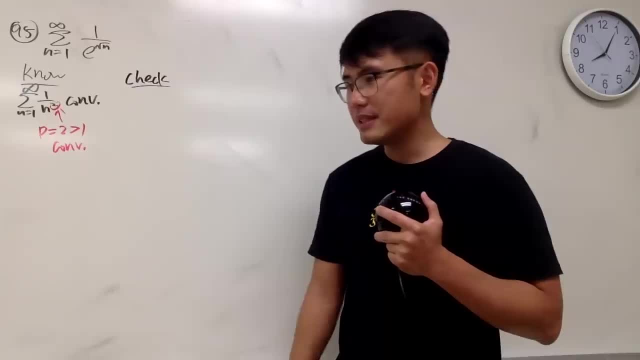 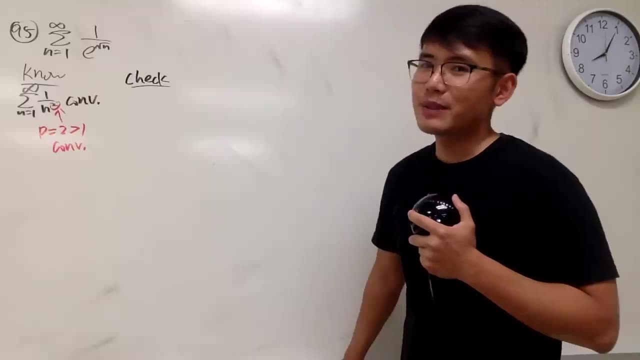 So I will just do a. Yeah, This is like the 1 and a half the square root of n, right? So I don't know. So, again, I don't want to just show you guys another version of the comparison test. 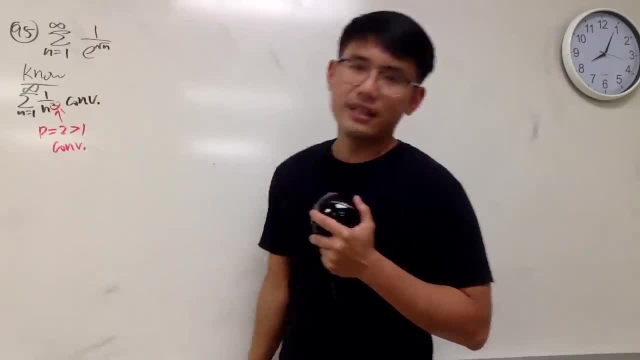 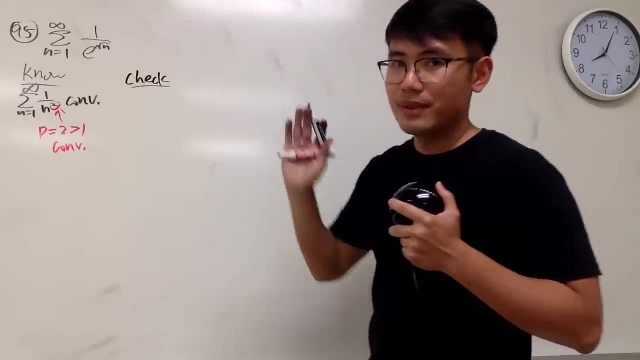 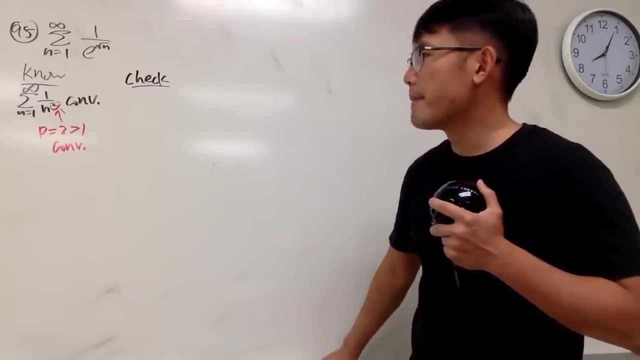 but just write it down seriously: Converges P-series. Thank god, Now we will do a real quick comparison. So this is just going to be a direct comparison. You will see You can also do a. Can I also do a limit? 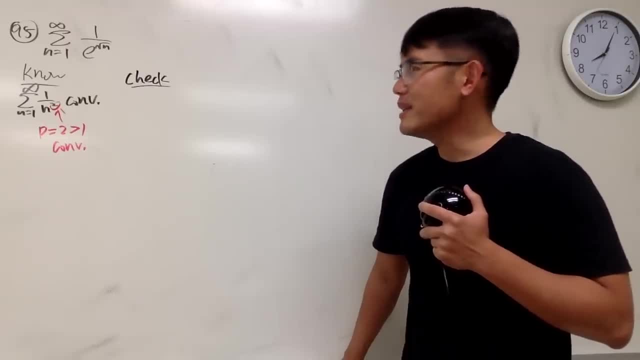 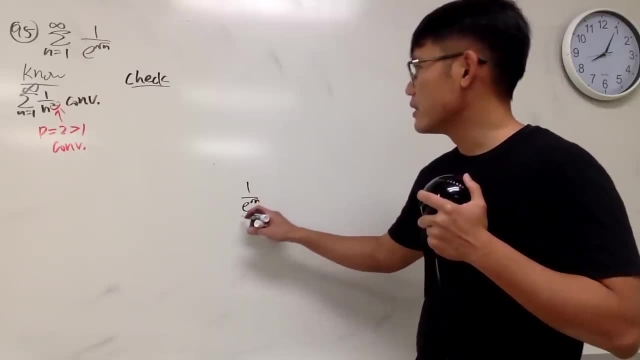 Why didn't I do a limit earlier? Yeah, why didn't I do a limit earlier? If I do a limit, computer design, Let me see 1 over e to the square root of n. Oh yeah, it's not going to be a nice value. 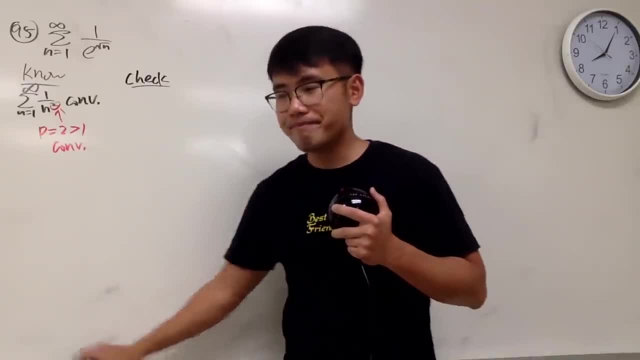 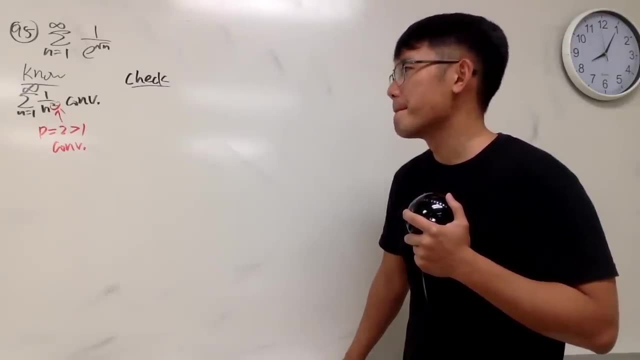 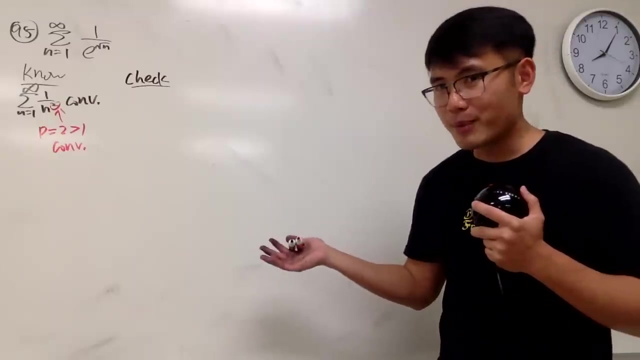 I have to take this as special case for that now. So I will just do a. Yeah, this is like the 1.5, the square root of n right Sigh, So I don't know. So again, I don't want to just show you guys another version of the comparison test. 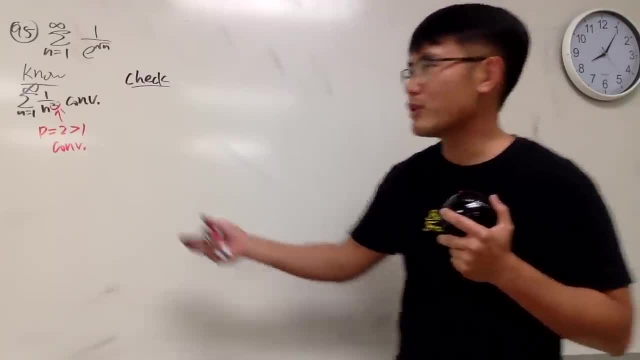 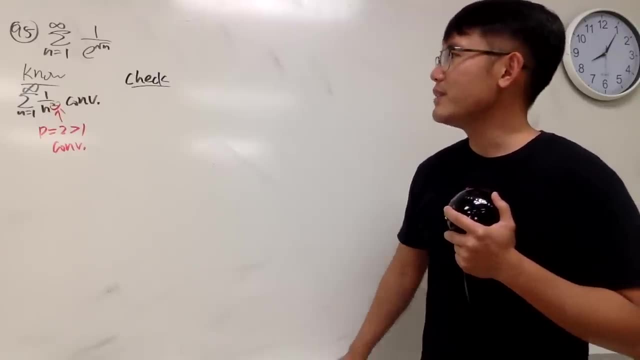 Sometimes, if you end up with 0 for the limit, you can actually draw a conclusion, but you have to pay attention to what kind of things that you know that you use right there. So let me not do that And let's see. if I don't use the comparison, what else can I do? 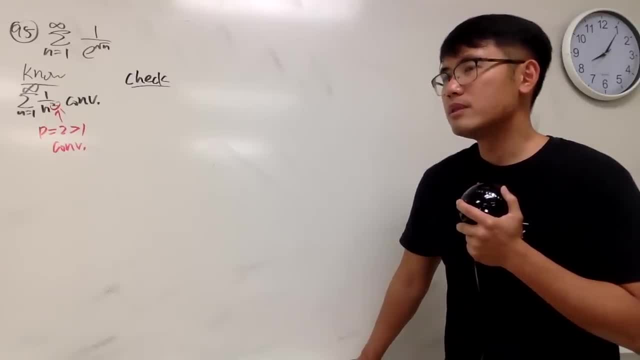 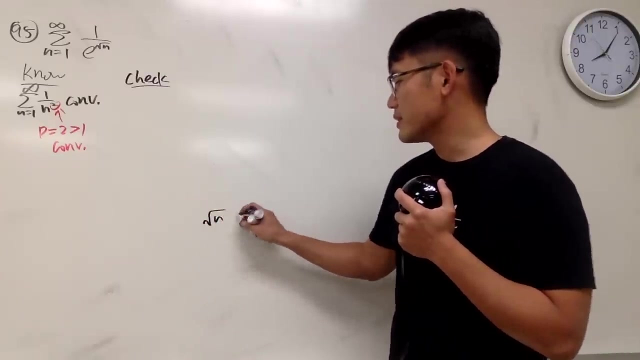 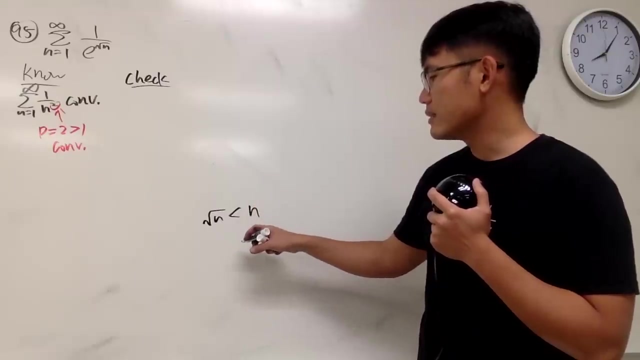 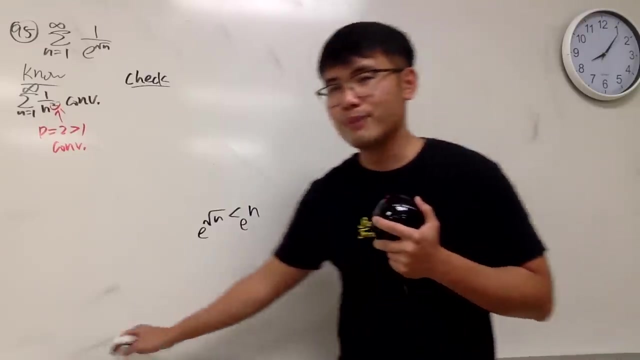 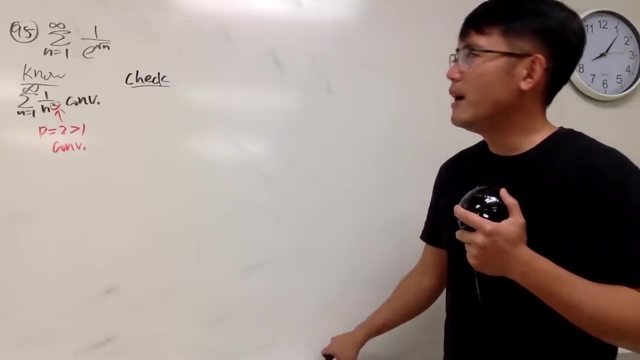 Integral test. Now, Hmm, What happens if I do the square root of n versus n? So this is smaller. This is that, Yeah, And into e. So like this: Oh man, No, Hmm, All right. 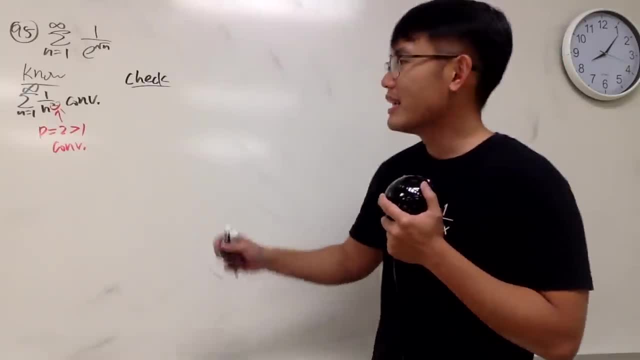 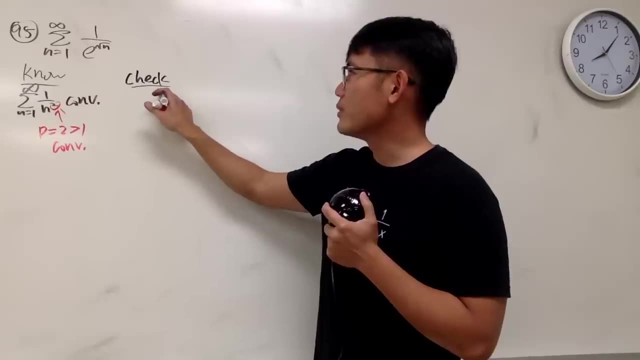 Let's see if you guys are okay with this approach, right? So again, I will use that, but I will do a direct comparison test, just like the one I was trying to do earlier. So I will put down the one that I want to find out. 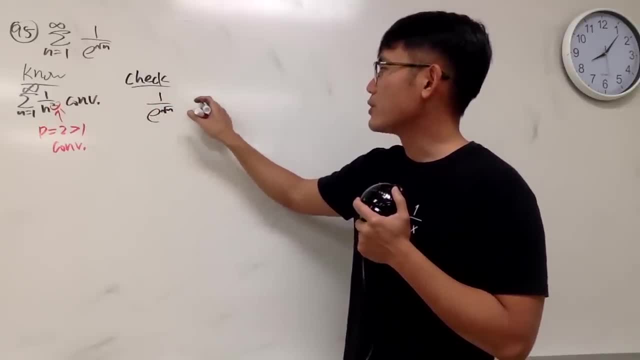 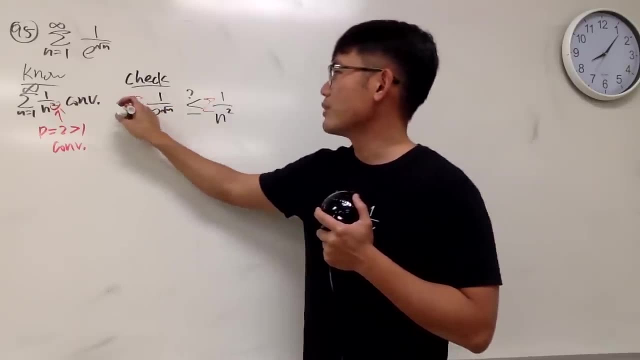 which is 1 over e, to the square root of n power. Okay, So if this is less than or equal to 1 over n squared, And if you guys know the deal, you should have the sum, and then you should also indicate that this is positive. 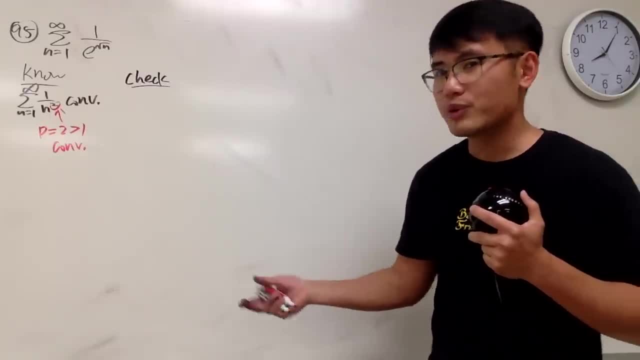 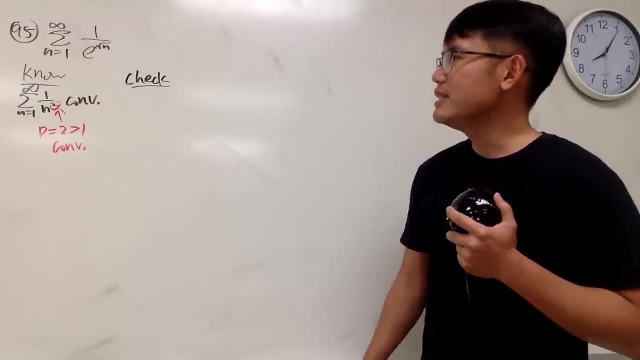 Sometimes, if you end up with 0 for the limit, you can actually draw a conclusion, but you have to pay attention to what kind of things that you know that you use right there. So Let me not do that And let's see. 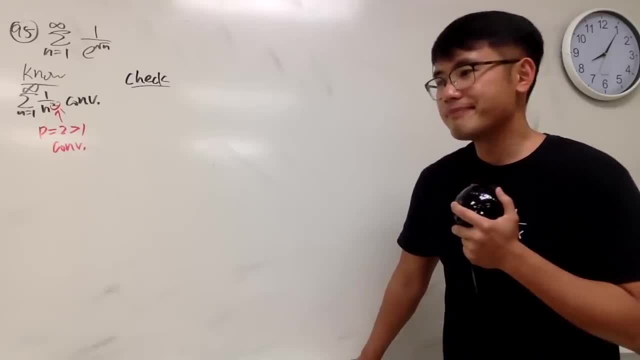 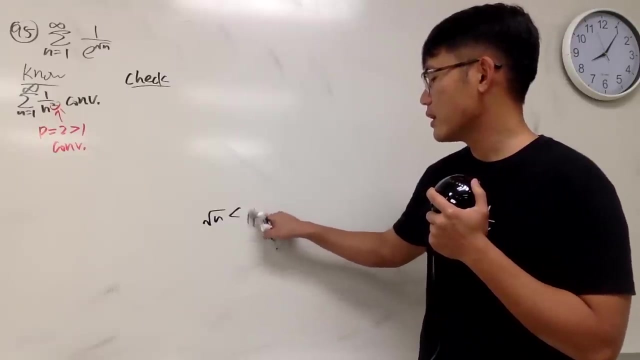 If I don't use the comparison, what else can I do? Integral test Now. Hmm, What happens if I do the square root of n versus n? So this is smaller, This is that, Yeah, And into e. So like this: 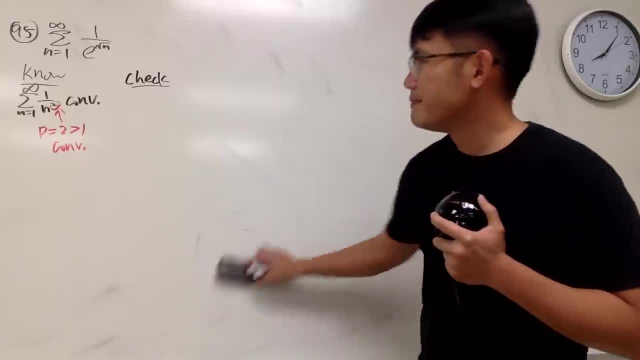 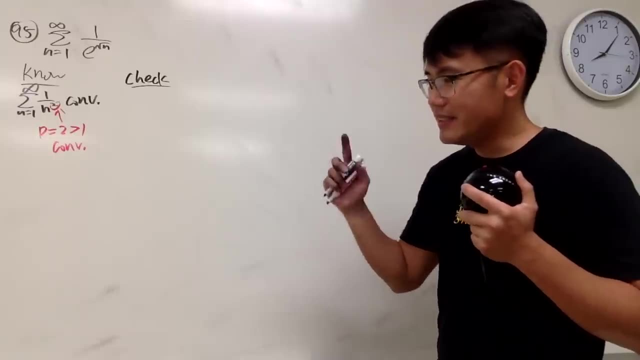 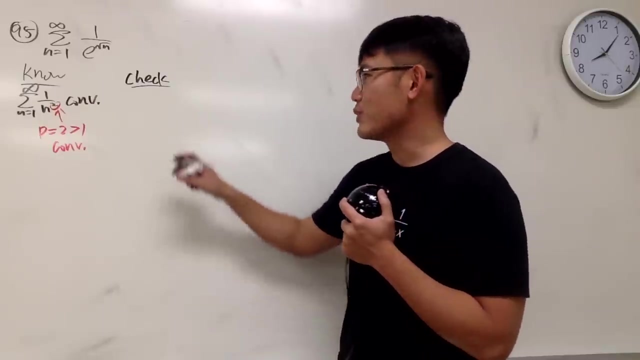 Oh man, No, Hmm, All right, Let's see if you guys are okay with this approach, right? So again, I will use that, But I will do a direct comparison test, just like the one I was trying to do earlier. 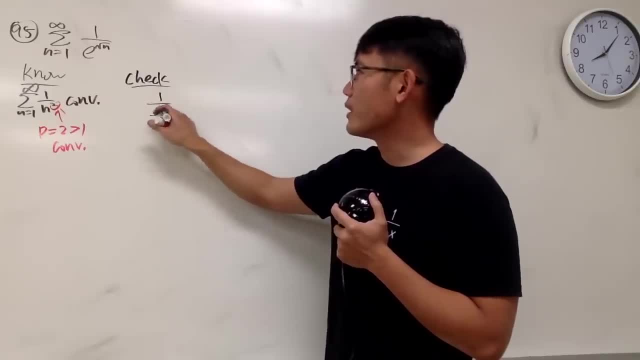 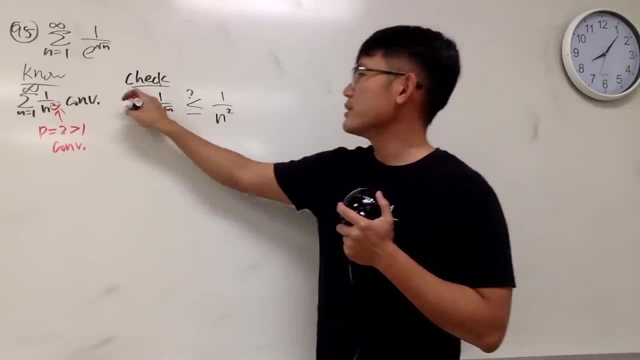 So I will put down the one that I want to find out, which is 1 over e to the square root of n power. I will show if this is less than or equal to 1 over n squared, And if you guys know the theory, you should have the sum. 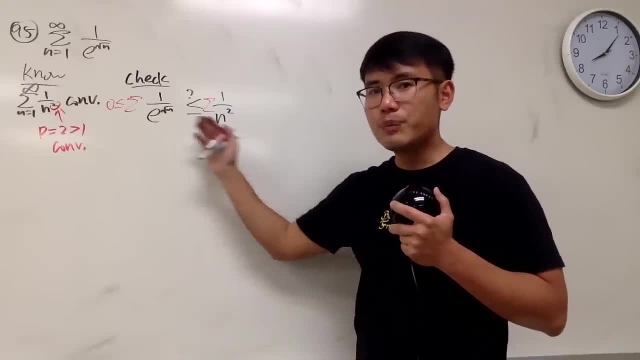 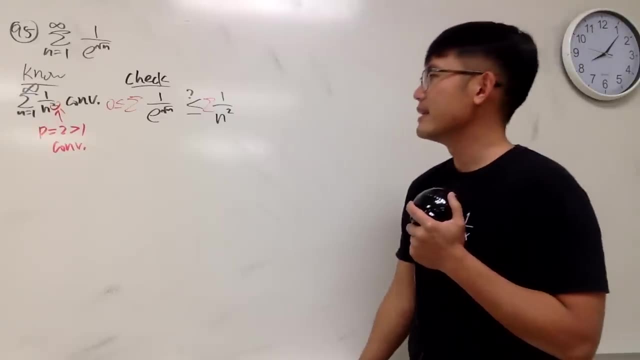 and then you should also indicate that this is positive And we put this down because this is a convergent. I will show that this is actually smaller than that, And Okay, So we just focus on this. 1 over e to the square root of n. 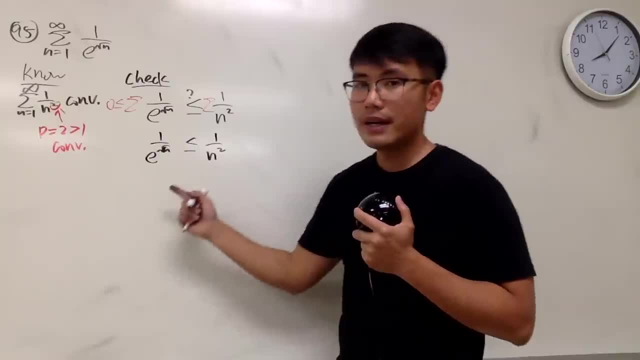 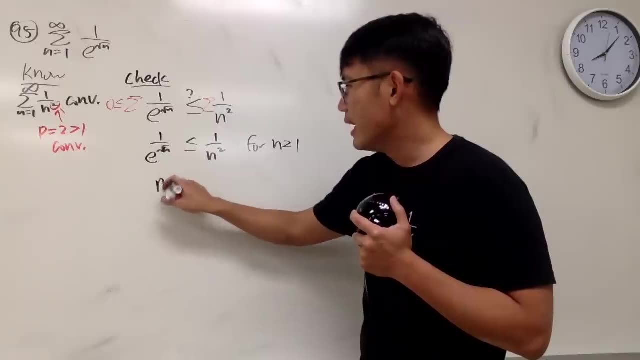 Less than or equal to 1 over Less than or equal to 1, over n squared right, And I want to see if this is true for n greater than or equal to 1.. Now here we go: Cross-multiply n squared less than or equal to e to the square root of n. 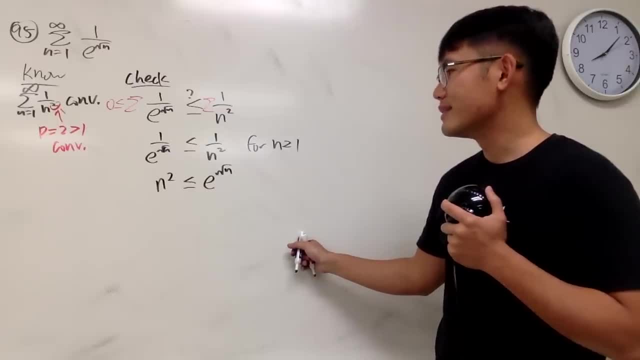 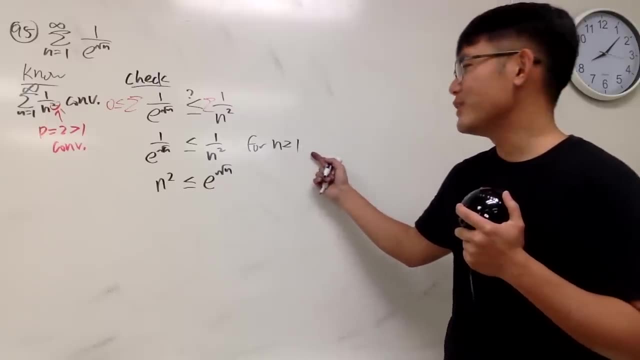 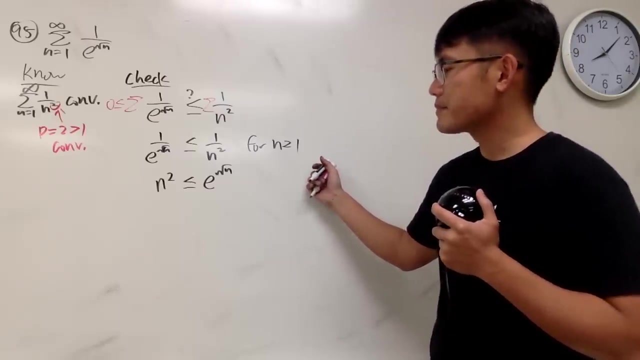 Like this: And if n is 1, works 2? 4? No, So again. so I didn't really fix this. I will just tell you guys that this is eventually true, right? Uh, Okay, I'll just. 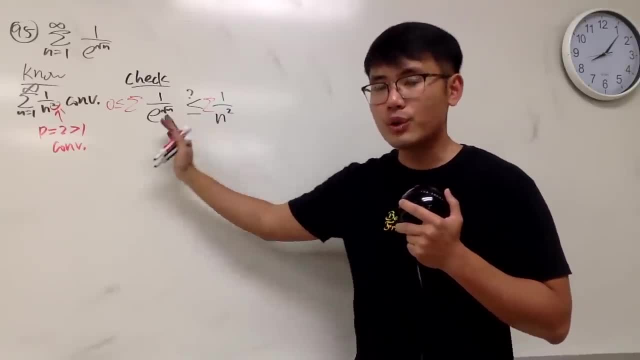 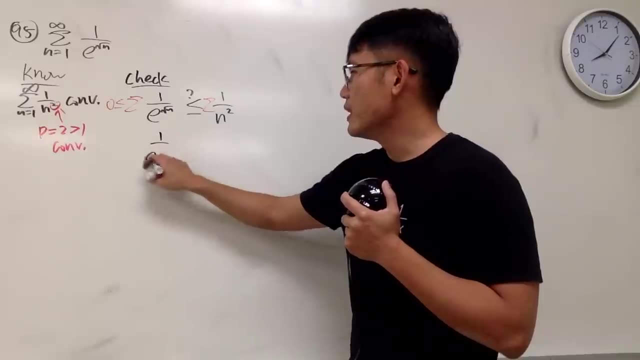 And we put this down because this is a conversion. I will show that this is actually smaller than that, And okay, So we just focus on this. 1 over e to the square root of n. less than or equal to 1 over n squared. 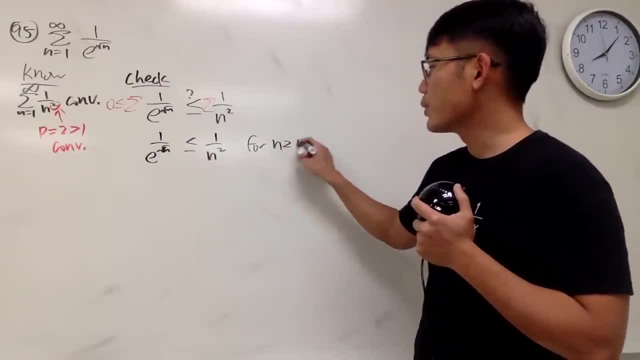 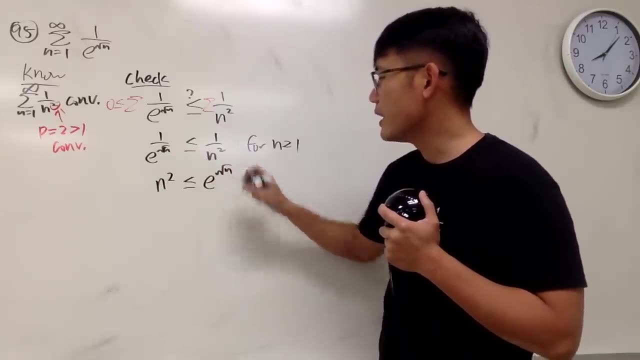 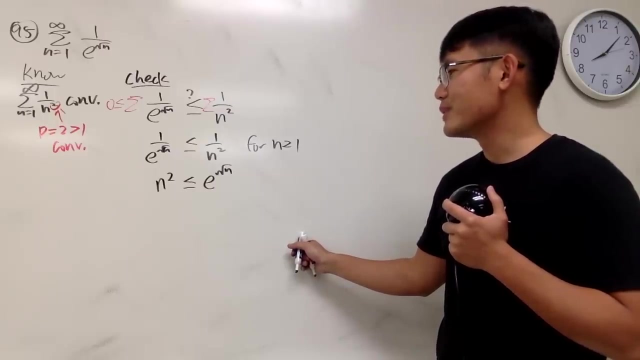 All right, And I want to see if this is true for n greater than or equal to 1.. Now here we go. Cross multiply n squared less than or equal to e to the square root of n, like this, And if n is 1, works 2 for no. 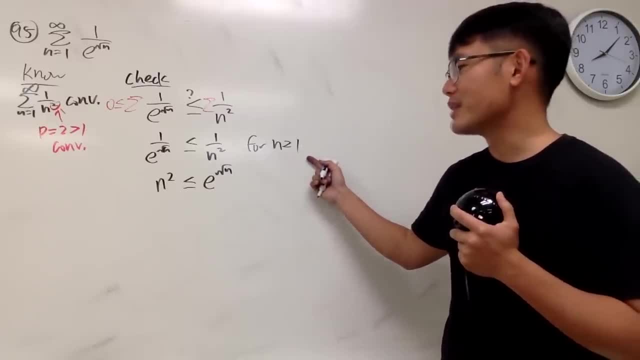 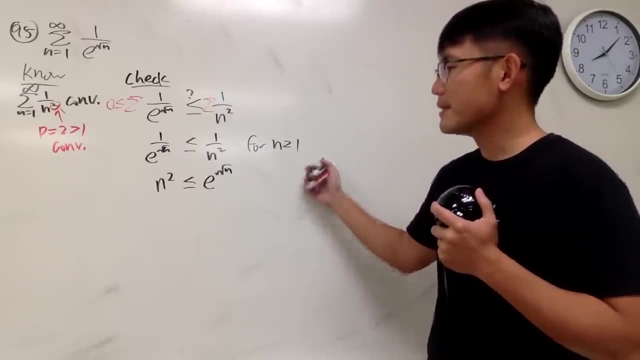 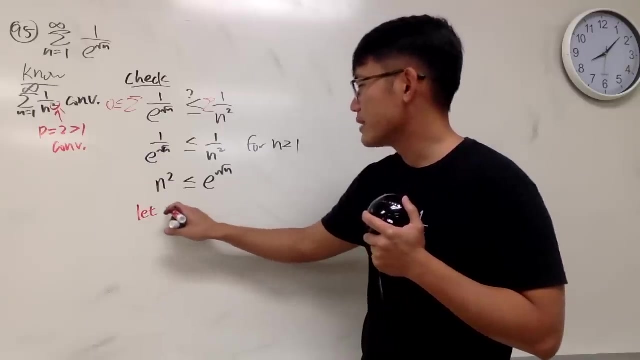 So again, so I didn't really fix this- I will just tell you guys that this is eventually true. All right, Okay, I'll just So. okay, I will just let Let's say: m Oh no. 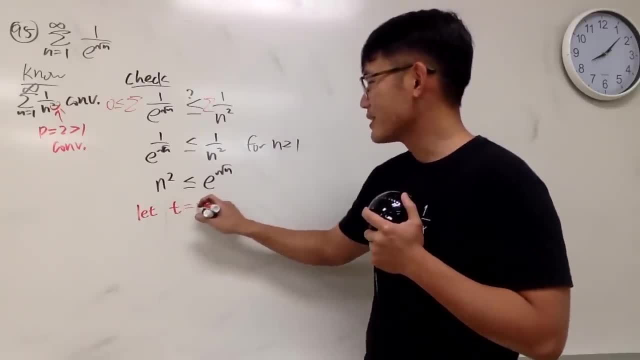 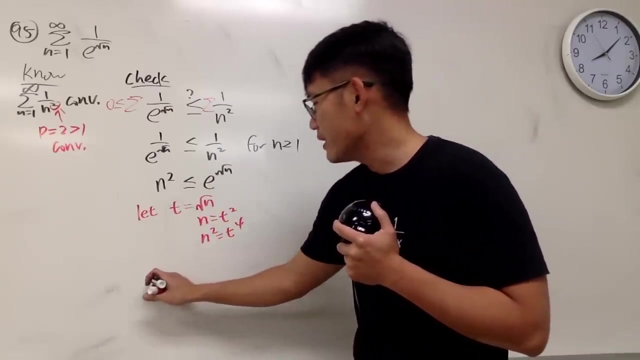 Let me just say, let's say t or something. t equals square root of n, So n is t squared. So n squared will be t to the fourth power. All right, So on the left-hand side you are comparing t to the fourth power. 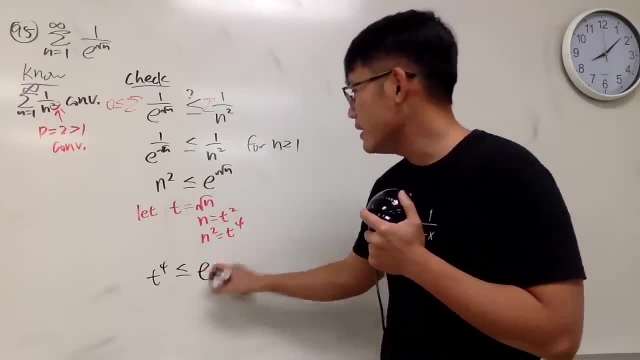 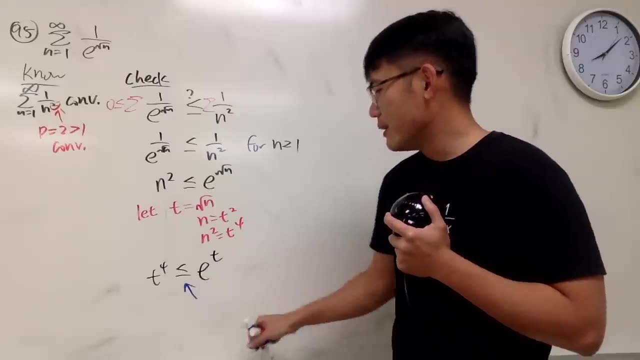 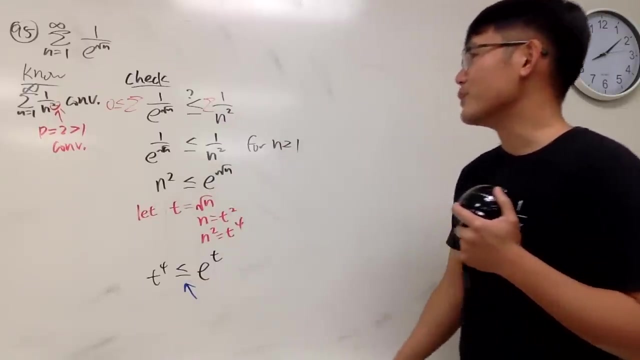 And on the right-hand side you have e to the t to the fifth power. So, as you can see, this right here is eventually true. So, but it's not true for n greater than 1.. So you have to kind of just pick the n value. 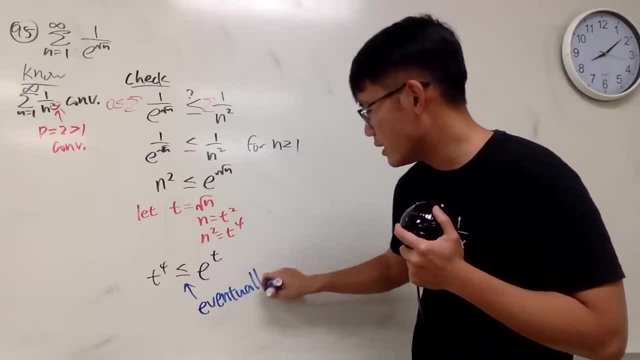 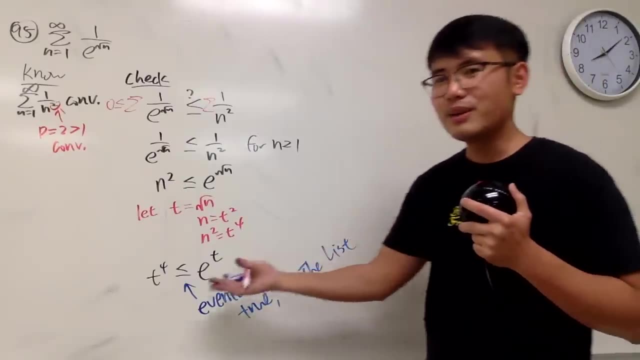 I will just tell you: eventually true by the list. So technically you can still do this. as long as this is eventually true, It doesn't have to be that n is equal to 1,, 2,, 3,, 4,, 5, and so on. 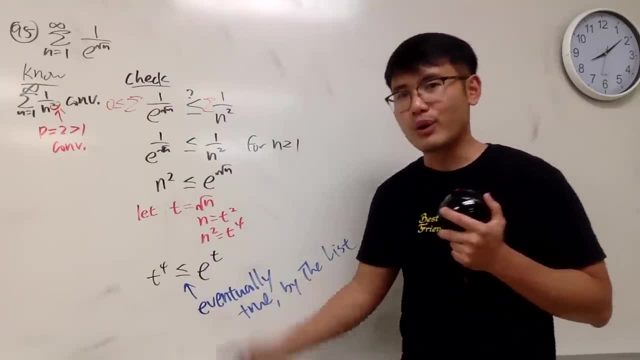 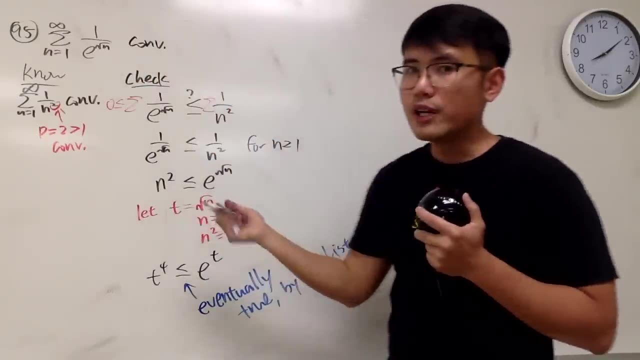 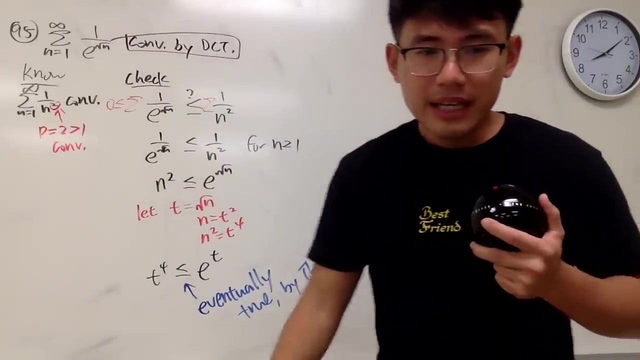 As long as This is true, after some n value, that's still okay, All right. But anyway, I will just probably tell you just this right here: This right here converges by direct comparison test. All right, So that will be it. 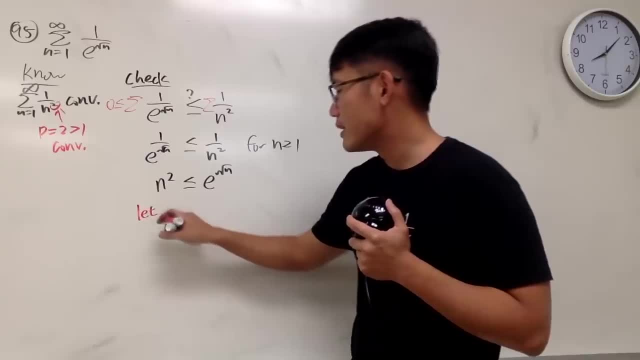 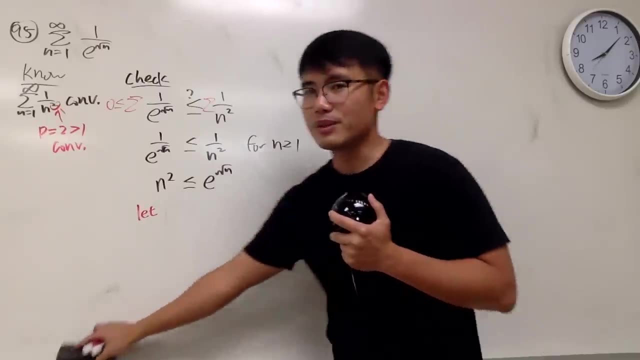 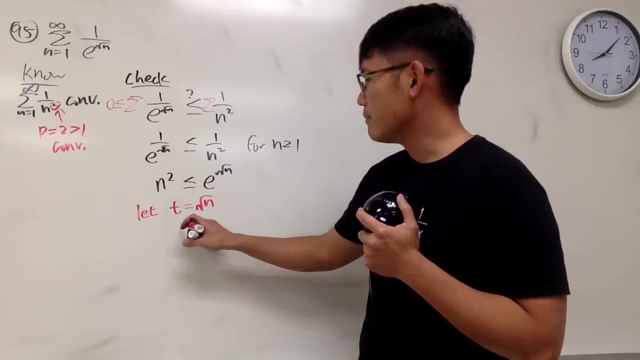 So Okay, I will just let Let's say Uh m, Oh no, Let me just say, let's say t or something. t equals square root of n, So, Um, n is t squared, So n squared will be t. to the fourth power. 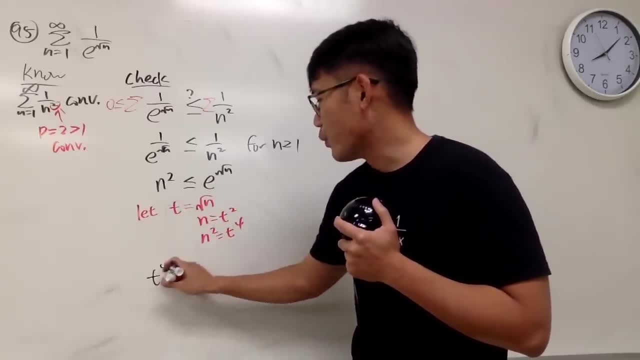 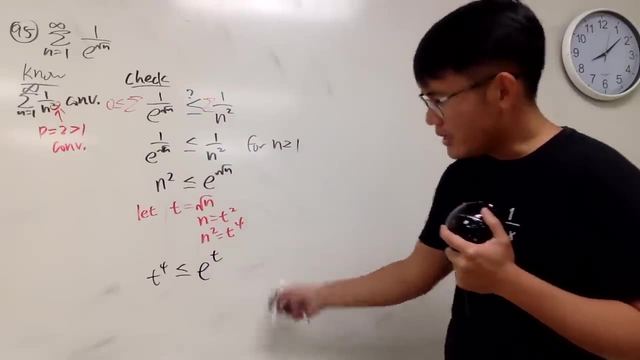 Right. So on the left-hand side you are comparing t to the fourth power And on the right-hand side you have e to the t's power. So, as you can see, this right here is eventually true So. 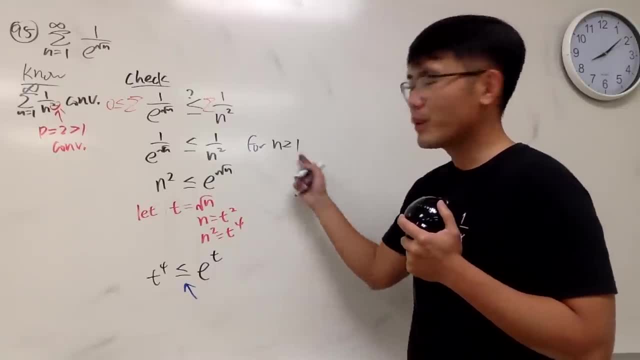 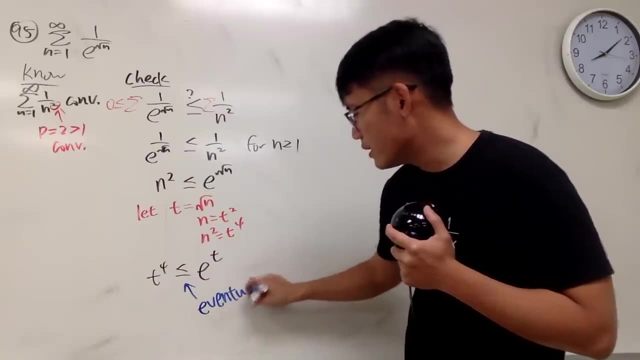 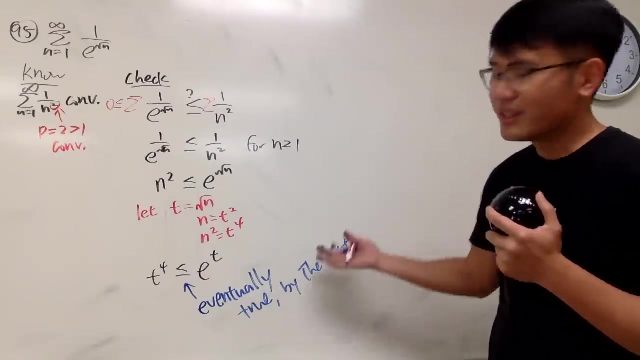 But it's not true for n greater than 1.. So you have to kind of just pick the n value, Right? I will just tell you eventually true by the list. So technically you can still do this as long as this is eventually true. 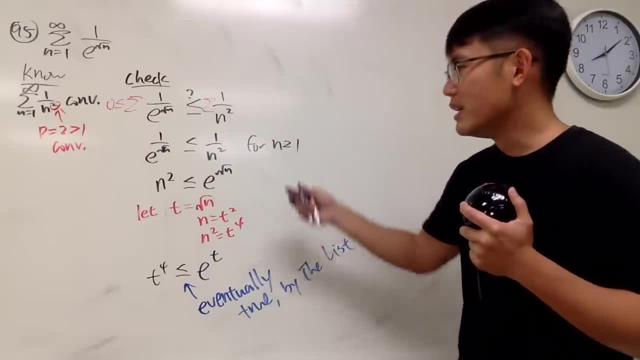 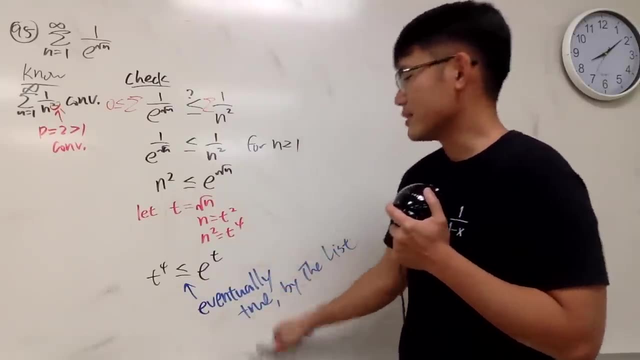 It doesn't have to be like n is equal to 1,, 2,, 3,, 4,, 5, and so on. As long as it's true after some n value, that's still okay, Right, But anyway, I will just probably tell you guys this right here. 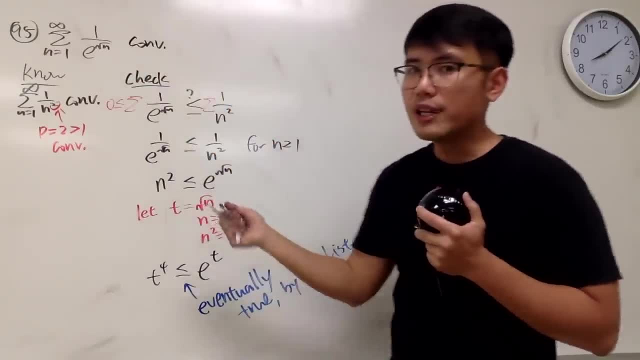 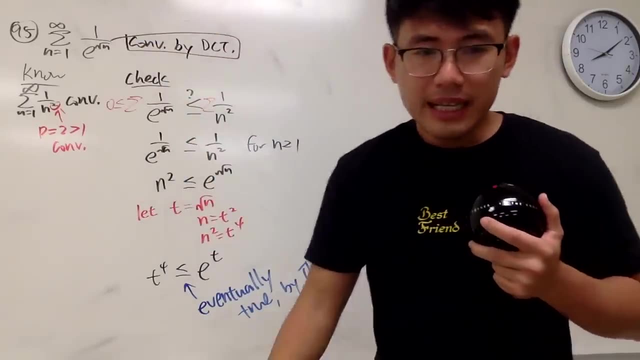 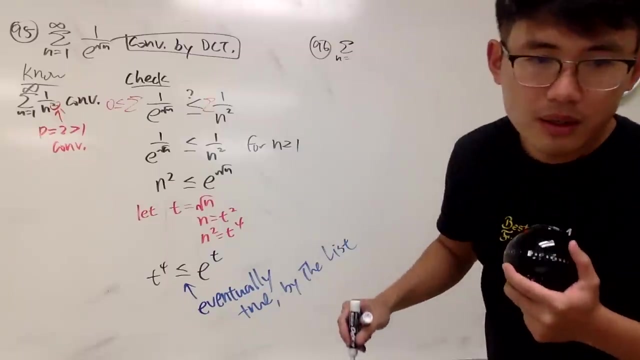 This right here converges by direct comparison test, Right? So that will be it, And just kind of do it on your own maybe, or something like that: 96.. 96.. The sum as n goes from 2 to infinity. 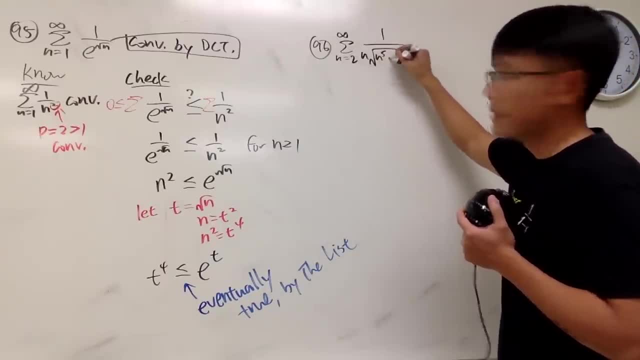 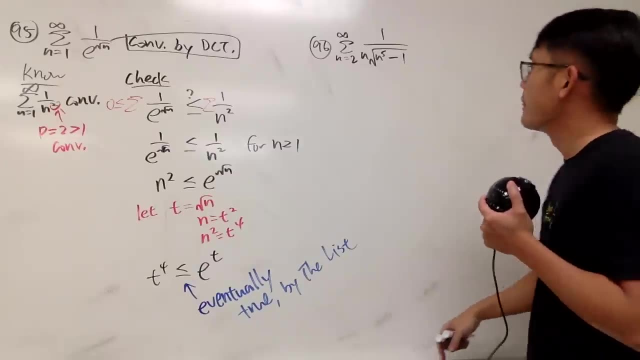 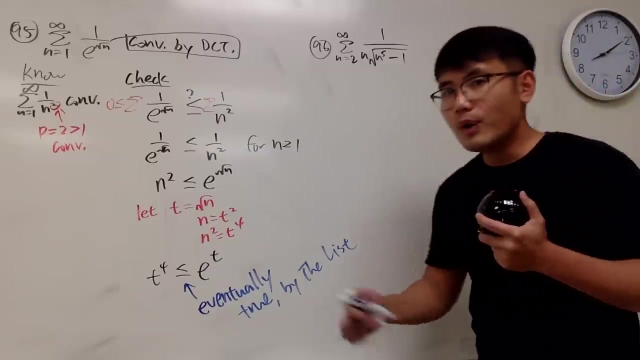 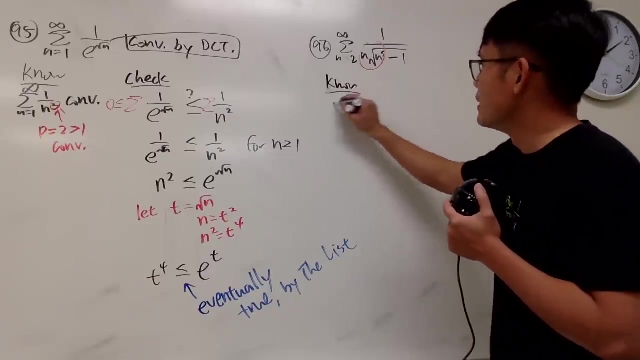 And we have 1 over n, square root of n to the 5. And we have minus 1.. Okay, Yeah, Something like that. Well, this right here is not that bad. Just do a limit comparison test Right, Write down what we know, which is the sum as n goes from 2 to infinity, 1 over this and that. 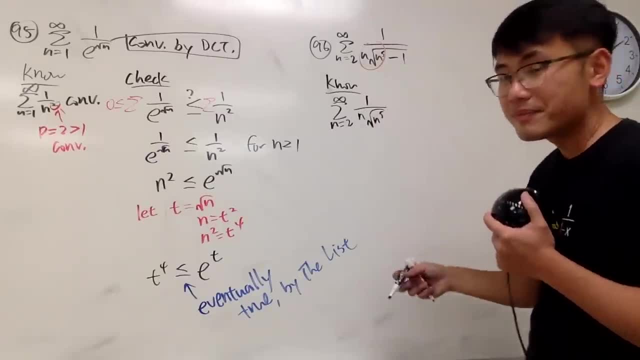 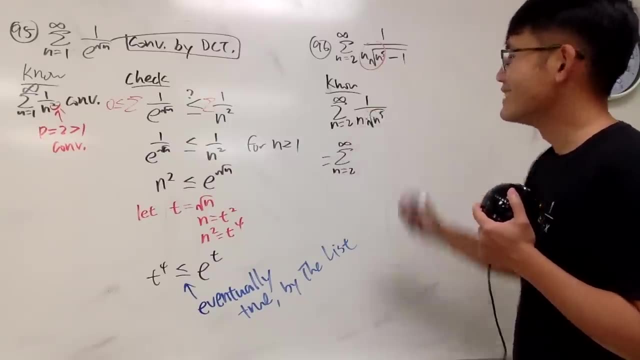 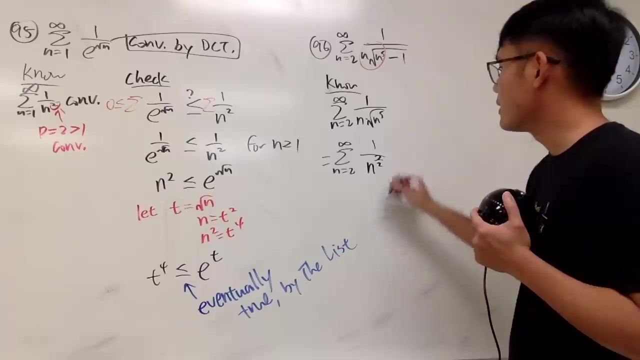 n and then square root of n to the 5, like this: Well, well, this is the sum, as n goes from 2 to infinity. This is n times that. So this is, I say n to the 5 over 2 power plus 1, which is 1 over n to the 7 over 2 power. 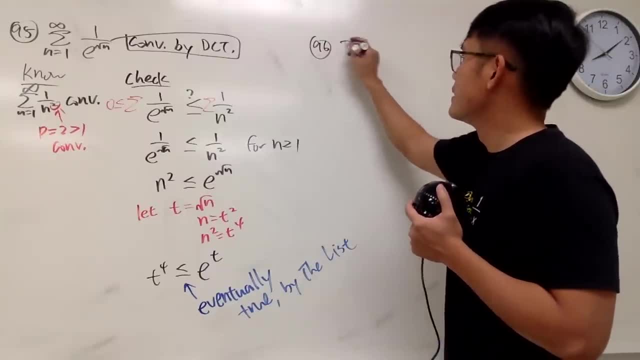 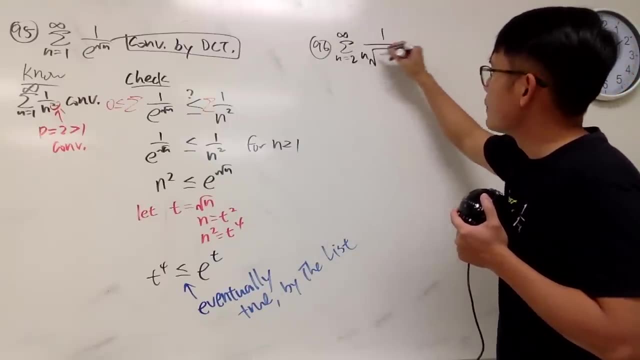 And just kind of do it on your own maybe, or something like that: 96.. The sum as n goes from 2 to infinity And we have 1 over n. squared root of n to the 5. And we have minus 1.. 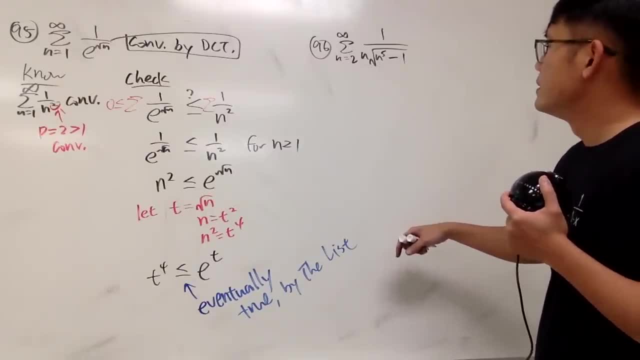 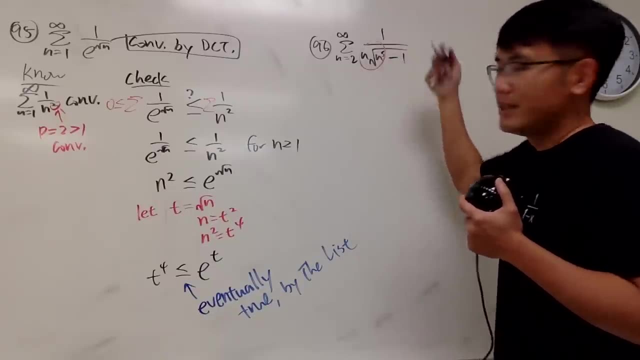 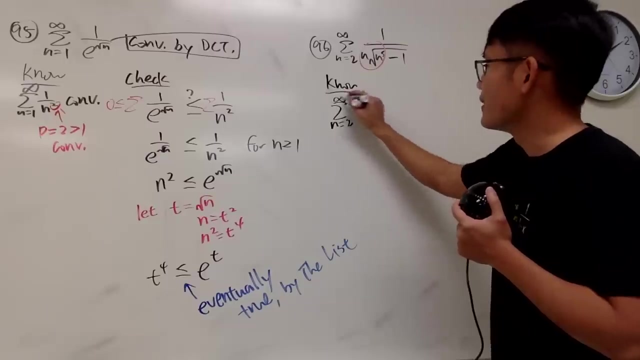 Okay, Yeah, Something like that. Well, this right here is not that bad. Just do a limit comparison test, right? So write down what we know, which is the sum as n goes from 2 to infinity, 1 over this and that n, and then square root of n to the 5, like this: 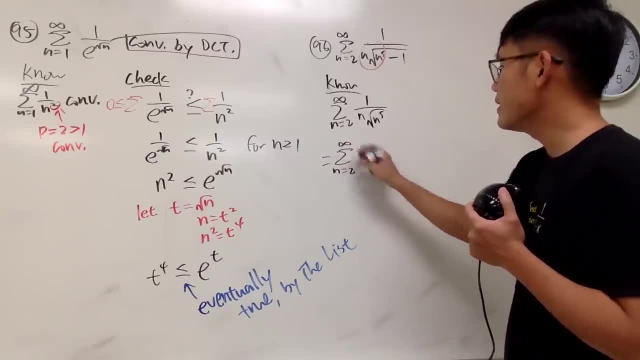 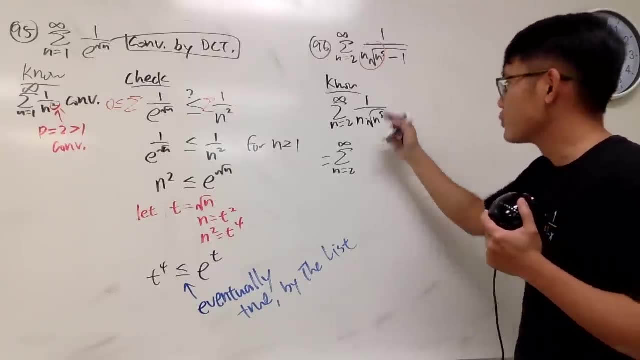 Well, well, this is the sum, as n goes from 2 to infinity. This is n times that. So this is: I say n to the 5 over 2 power plus 1, which is 1 over n. to the 7 over 2 power. 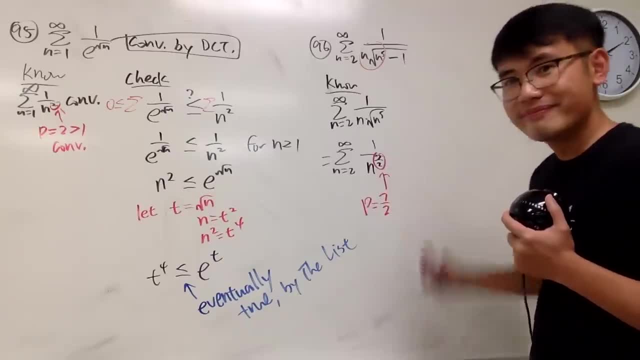 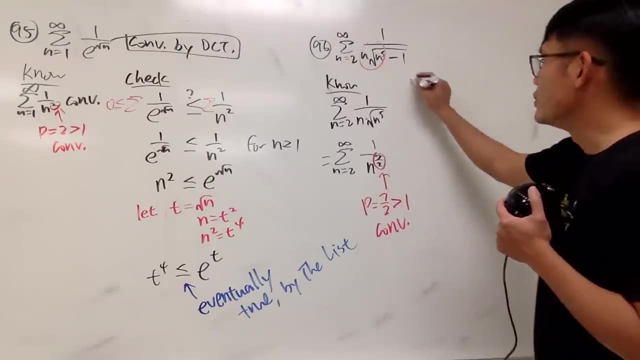 So this right here p is 7 over 2, which is greater than 1, which means this right here converges, so that when we check, we can just do this real quick. You get this real quick, guys. I'll put this down real quick. 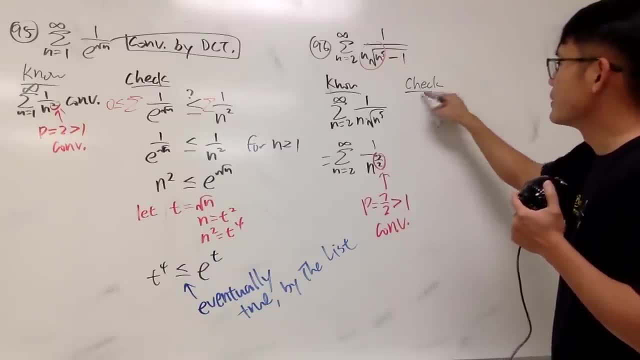 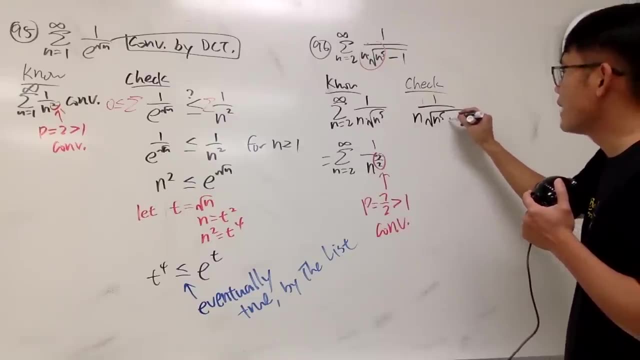 We get the limit comparison test which is 1 over n times. okay, this is not like n's root n times the square root of n to the 5 minus 1 over this guy, because I can cancel the n nicely: n to the 5, like that. 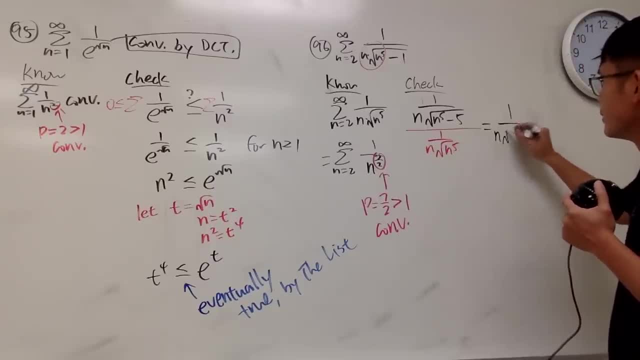 And then, of course, you do the reciprocal. So this is the usual thing, right? So you should be able to do all this by now already. n to the 5. Over: 1. Cancel, cancel, and oh why. 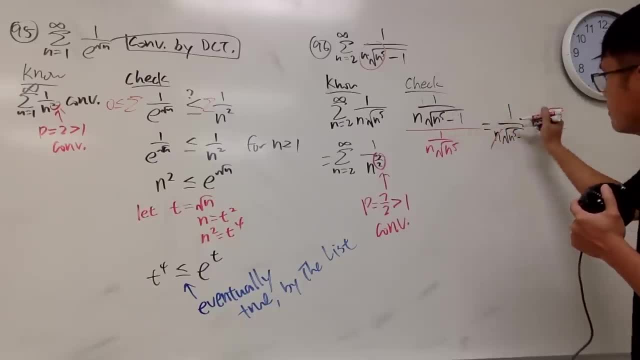 This is just minus 1.. Minus 1, right. Minus 1, minus 1.. Anyway, take a look at that and that and this right here will be just going to approach 1.. That's nice. This is greater than 0, so we can draw a conclusion. 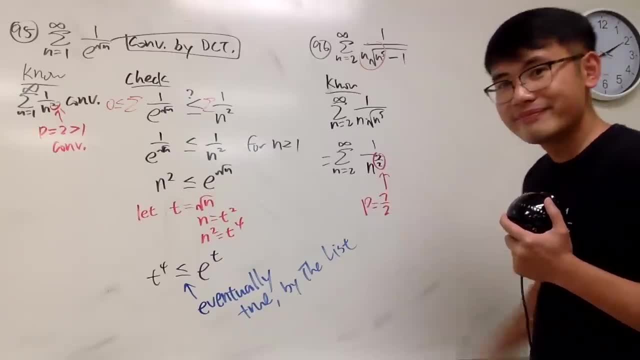 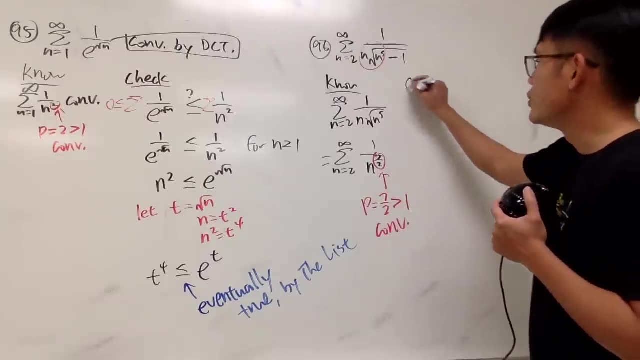 So this right here, p is 7 over 2.. Which is, Which is greater than 1, which means this right here converges, so that when we check, we can just do this real quick. You get this real quick, guys. 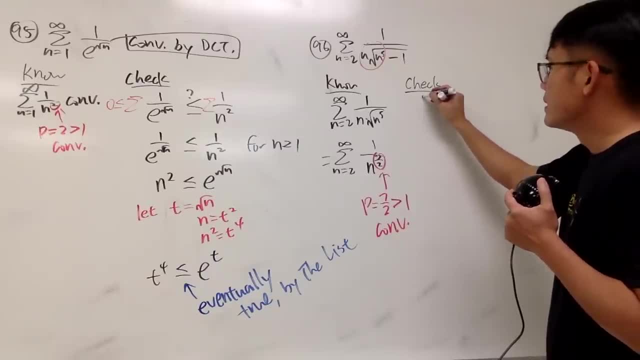 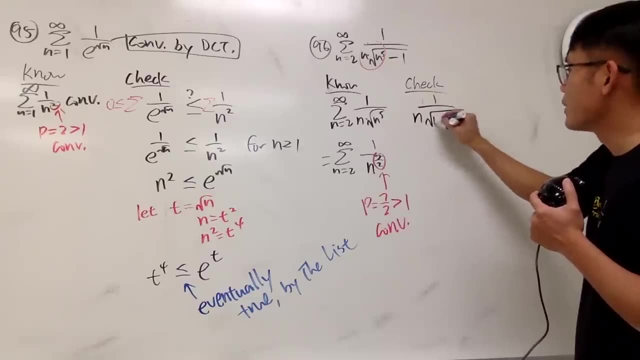 I'll put this down real quick. We get the limit comparison test, which is 1 over n times. okay, this is not like n's root n times the square root of n to the 5 minus 1 over this guy, because I can cancel. 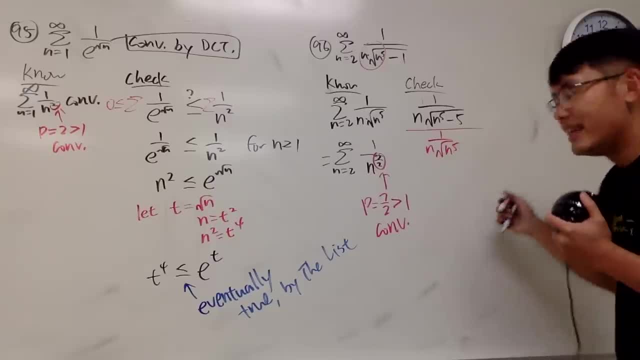 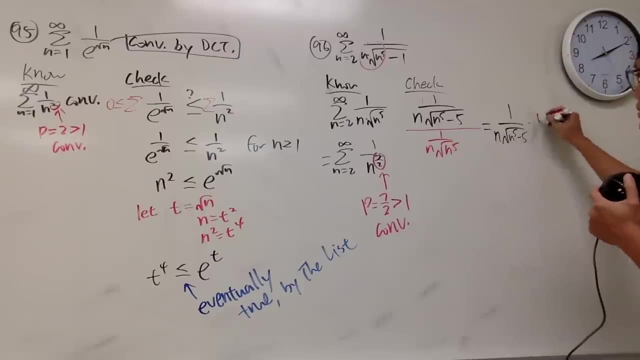 the n nicely. n to the 5, like that. And then of course you do the reciprocal. so this is the usual thing, right? So you, just you should be able to do all this by now already. n to the 5 over 1.. 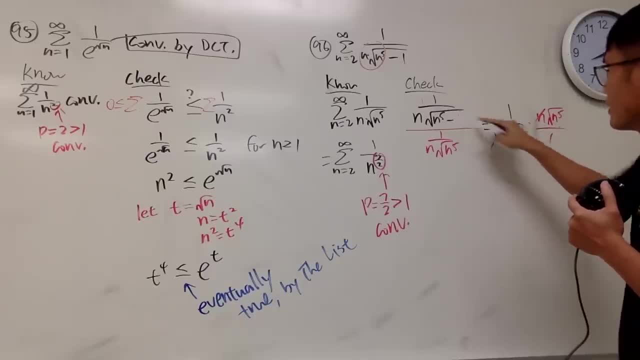 Cancel, cancel and oh why? This is just minus 1.. Minus 1, right. Minus 1, minus 1.. Anyway, take a look at that and that and this right here will be just going to approach 1.. 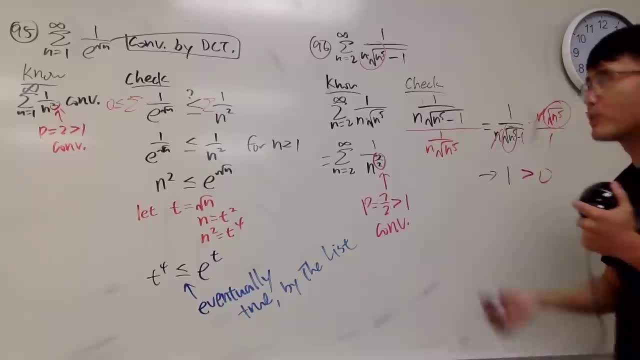 That's nice. This is greater than 0, so we can draw a conclusion: Yay, Okay, so this right here converges right, because this was convergent as well by limit comparison test. So this is very, very nice. 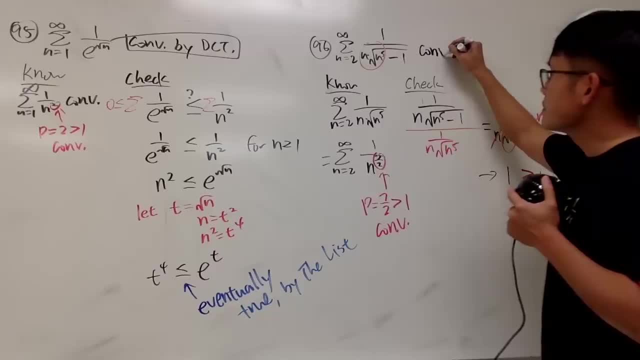 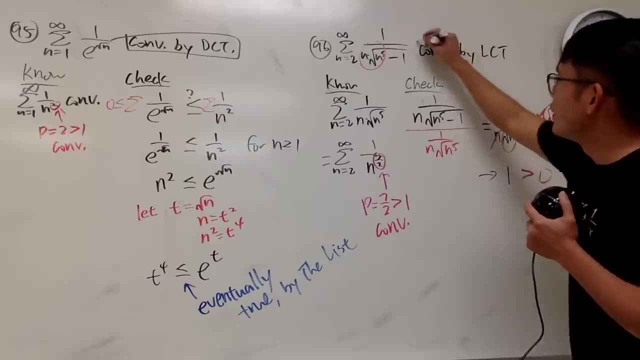 Yay, Okay, so this right here converges- right, because this was converging as well- by Limit, complete and test. So this is very, very nice. Okay, you guys excited, You guys excited. Oh, my God man. 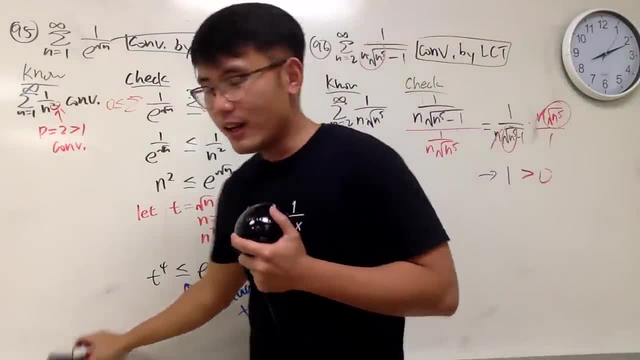 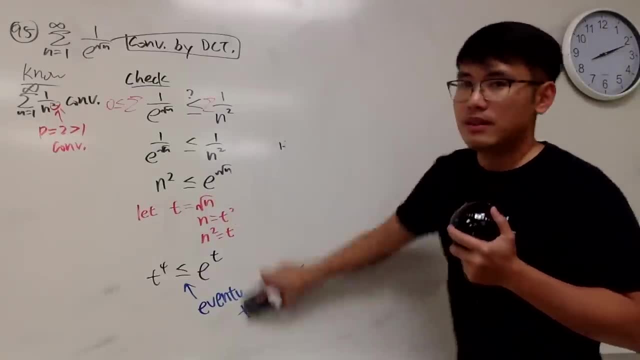 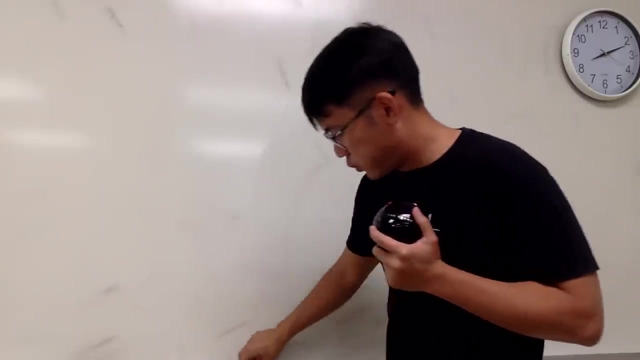 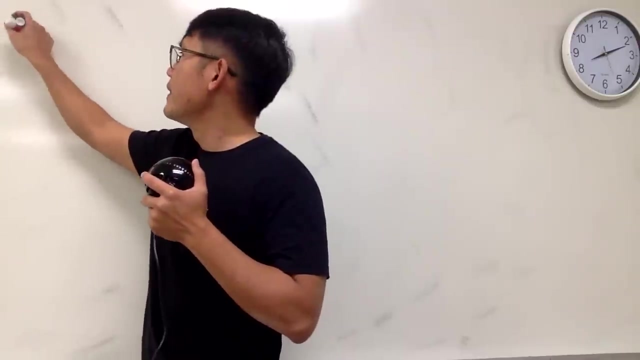 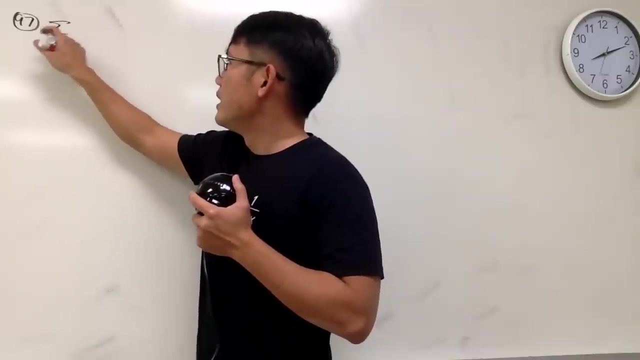 Okay, you guys excited, You guys excited. Oh my god man, Oh my god. Let's see if I can fill in the rest of the questions. all right here. I don't know, though, Number 97. Okay, Okay, this is going to be more than the integral video, but it's okay. 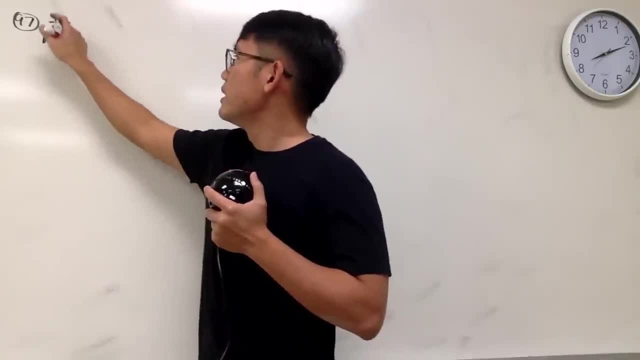 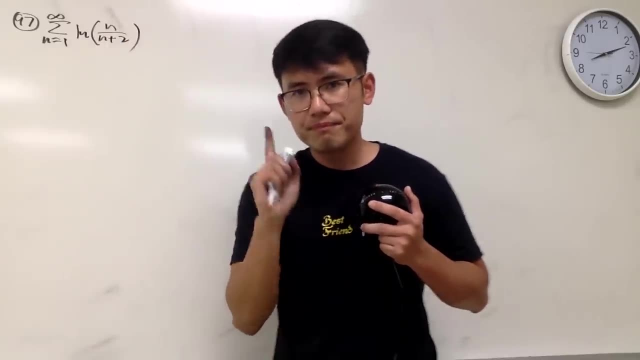 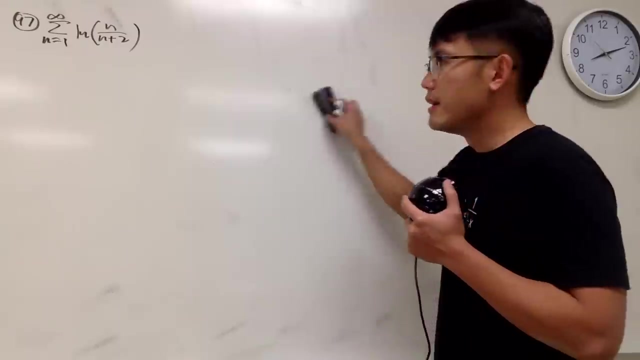 n goes from 1 to infinity And here we have natural log of n over n plus 2.. Now if you let n goes to infinity and do the n to infinity, you're going to get n to infinity. If you let n goes to infinity and do the n, if you do the, what's that test for divergence? 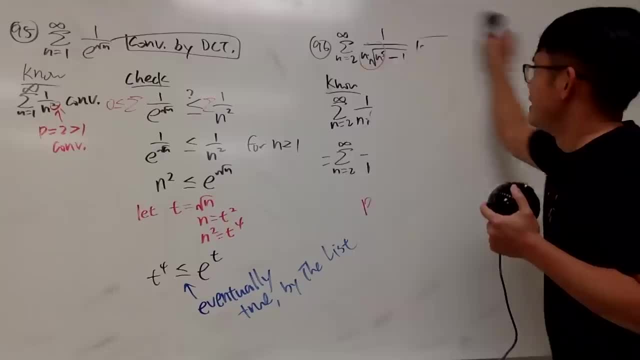 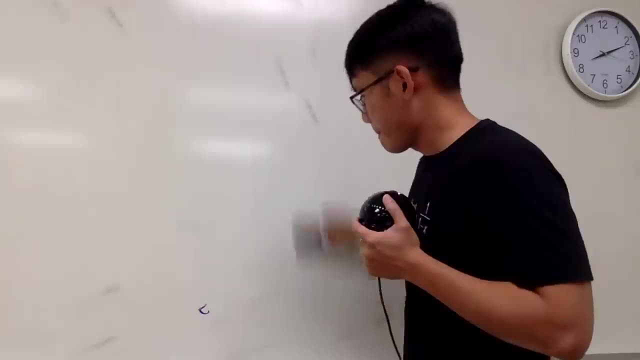 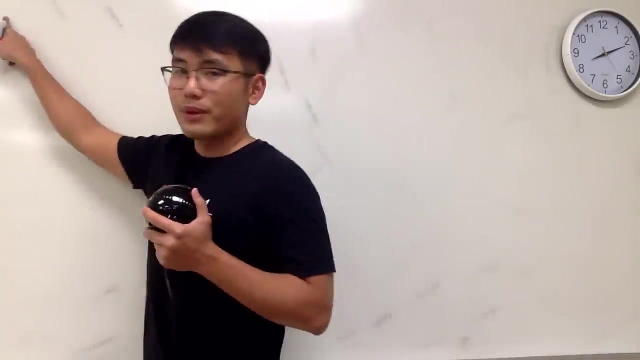 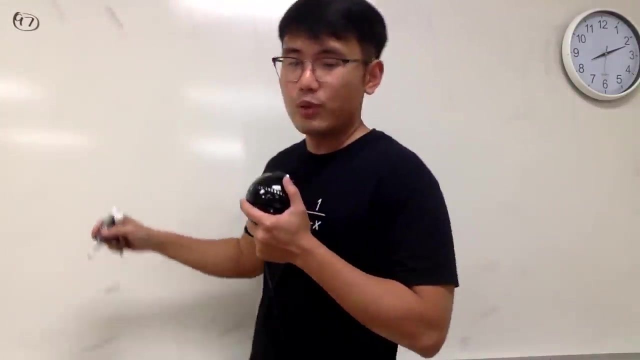 Oh, my God, Let's see if I can fill in the rest of the questions. all right here, I don't know. Number 97.. Okay, this is going to be more than the integral video, but it's okay. n goes from 1 to infinity. 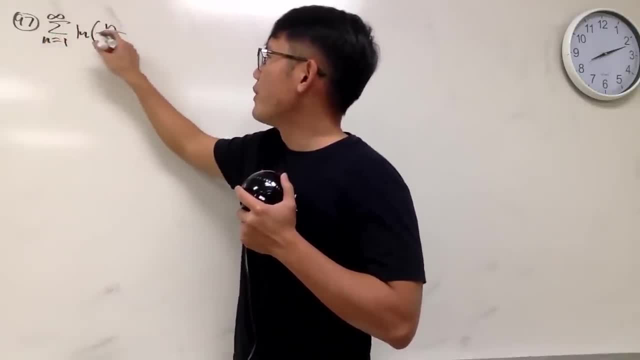 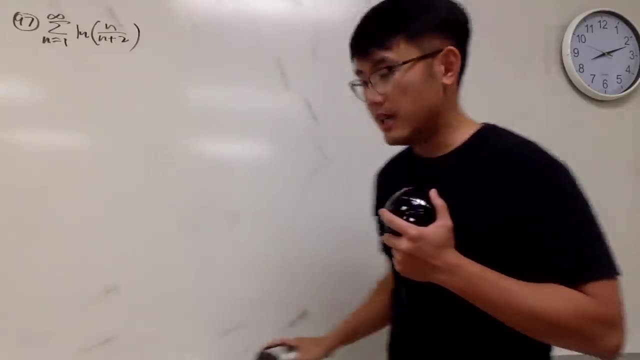 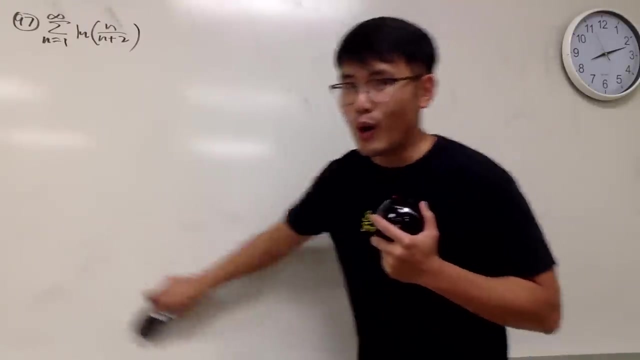 and here we have natural log of n over n plus 2.. Now, if you let n goes to infinity and do the n's, if you do the, what's that Test for divergence? No, because inside you get 1, right. 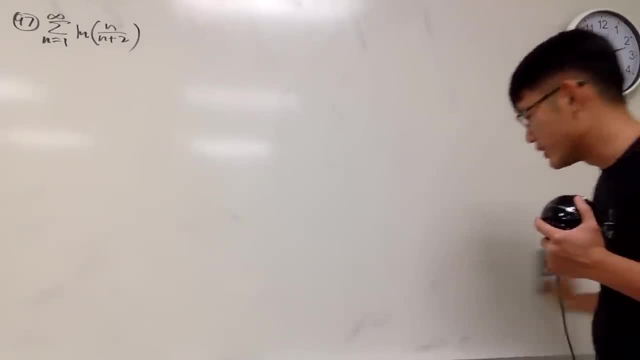 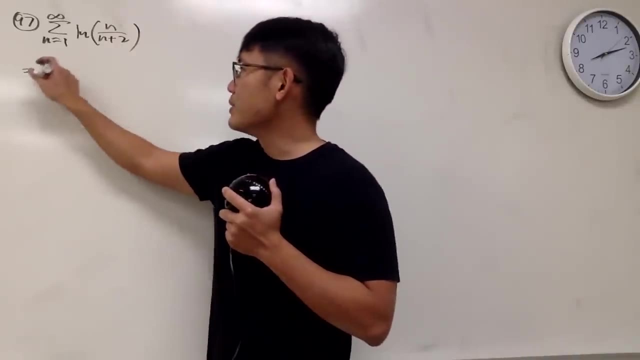 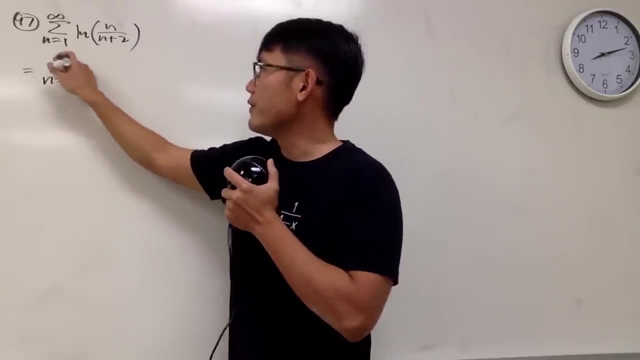 Okay, and then ln 1 is 0, so the truth is, we cannot use the test for divergence for this. But don't forget this right here is actually the same as the sum. okay, the sum as n goes from 1 to infinity, and here we have ln of n and then minus ln of n plus 2.. 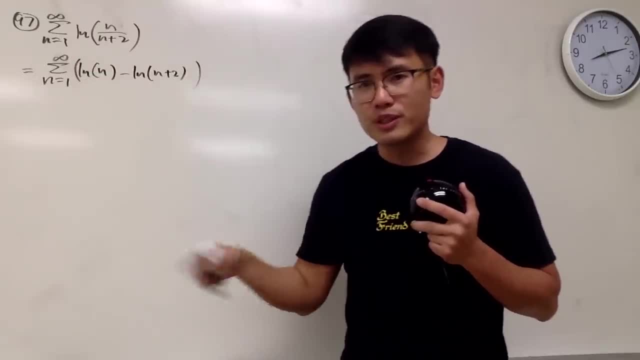 And notice they are actually of the same time or just off by 2.. So this is actually just a geometry, Okay. Okay, Just a telescoping series. So let's see if we converge this or not. All right, 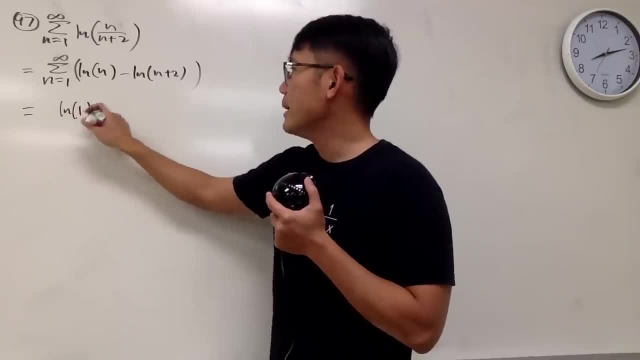 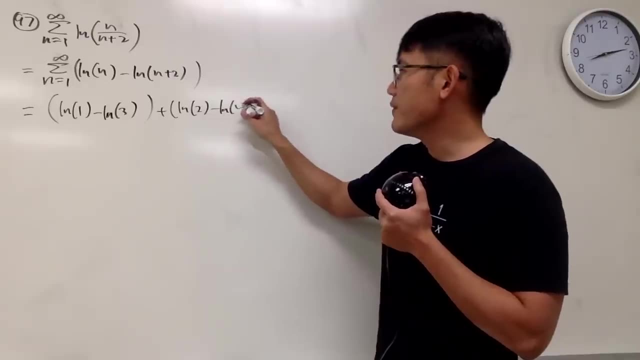 So this right here: if you put in 1,, so you have ln 1 minus ln 3, and then plus ln 2 minus ln 4.. Let's do it this way Now. let's do it this way. 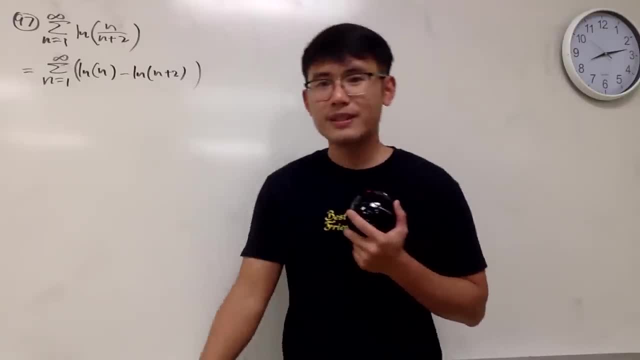 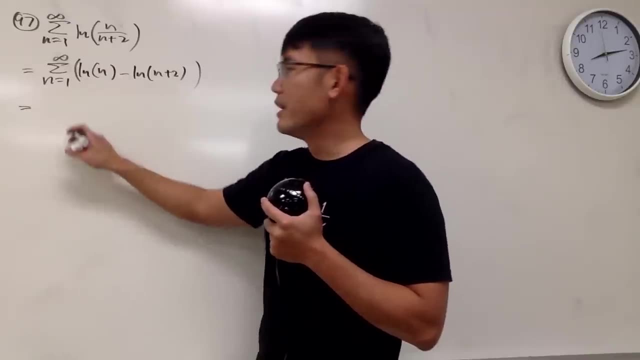 I'll show you the quick way to do this Quick way to do this. Okay, here we go. This is off by 2.. So we're just plotting the first two. So we're just plotting the first two numbers. 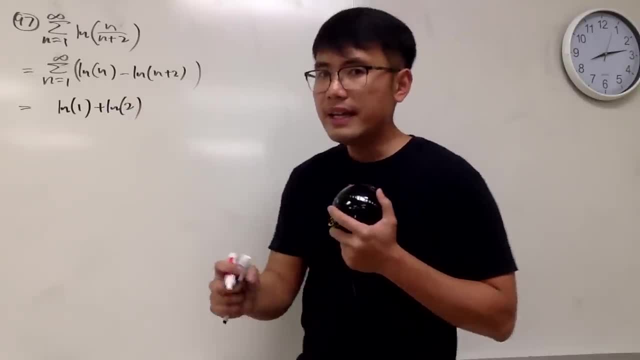 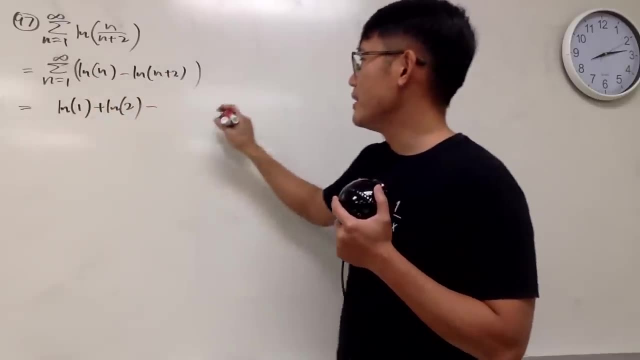 In other words, we get ln 1 plus ln 2, all right. and then you're going to subtract. The first term is going to get cancelled, cancelled, right. So this is going to be the last term, right, ln of n plus 2.. 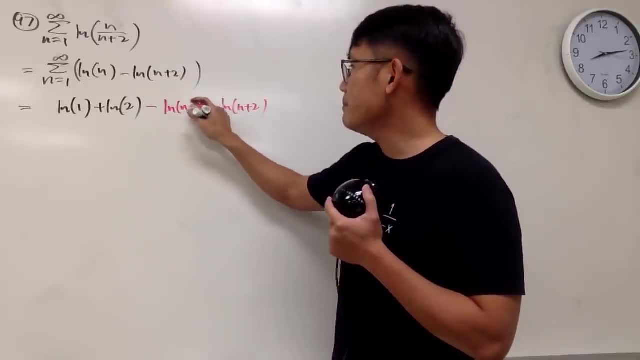 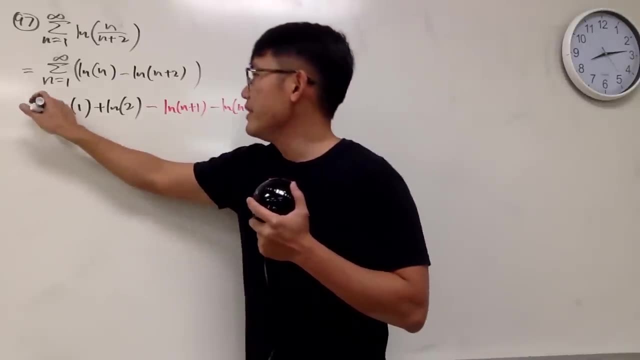 And then you also have to put on another term before that, so it's ln of n plus 1. That's it, Okay, seriously, Two things in front, two things in the back, and then you take the limit, and this is the. 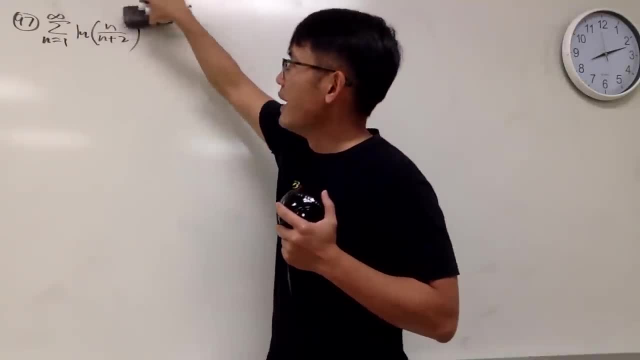 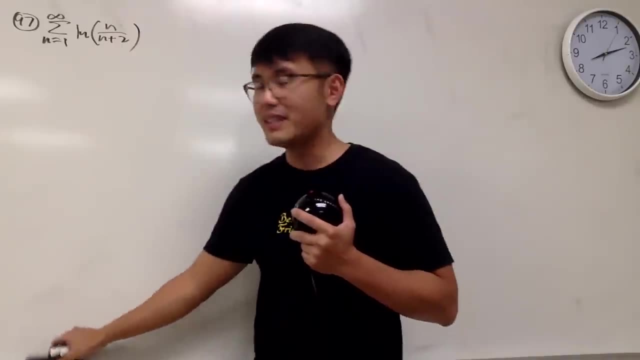 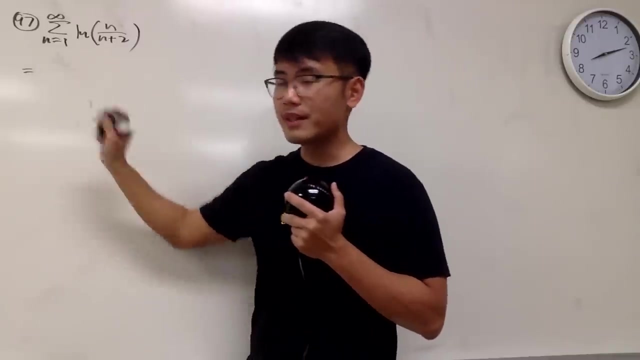 No, because inside you get 1, right, and then ln 1 is 0. So the truth is, we cannot use the test for divergence for this. But don't forget this right here is actually the same as the sum. okay, the sum as n goes. 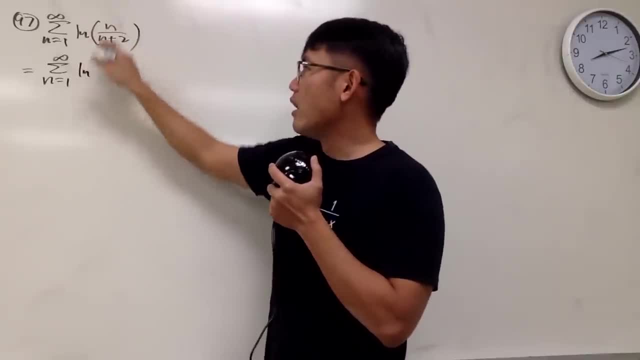 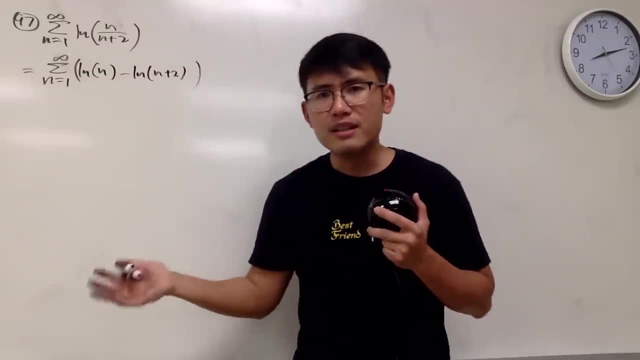 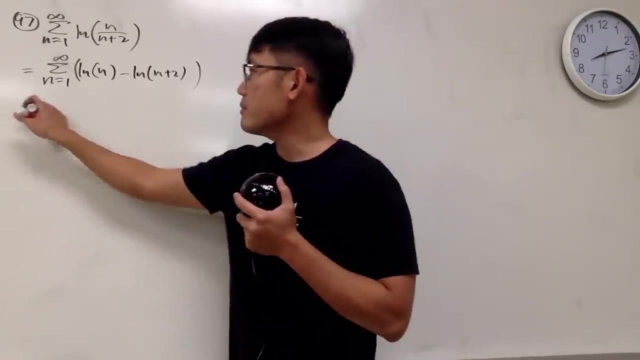 from 1 to infinity. And here we have ln of n and then minus ln of n plus 2. And notice they are actually of the same kind or just off by 2.. So this is actually just a telescoping series. So let's see if we converge this or not. all right, 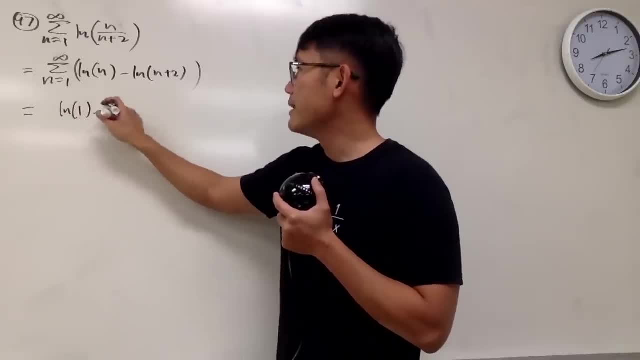 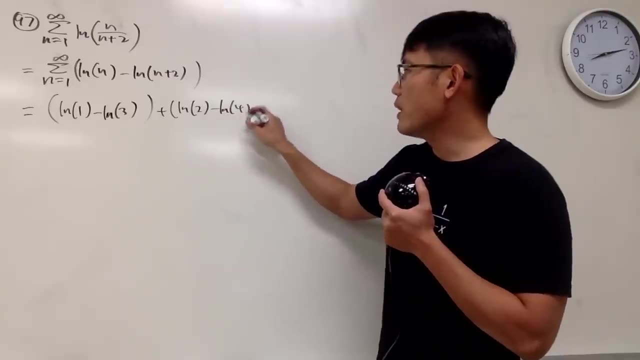 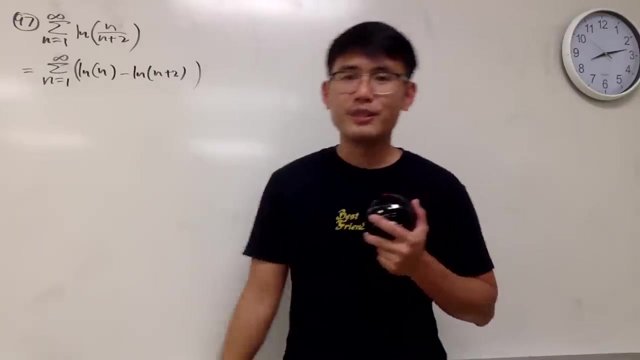 So this right here, if you put in 1, so you have ln 1 minus ln 3, and then plus ln 2 minus ln 4.. Then let's do it this way. Now, let's do it this way. I'll show you the quick way to do this quick way to do this. 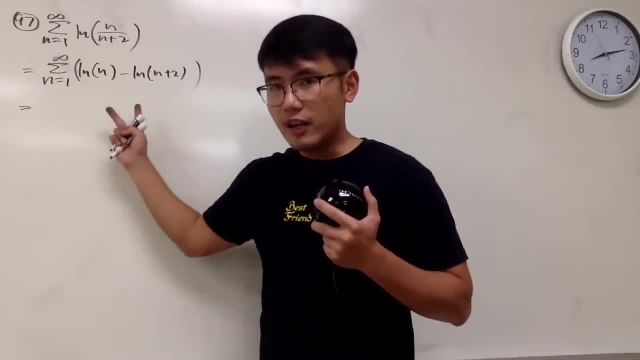 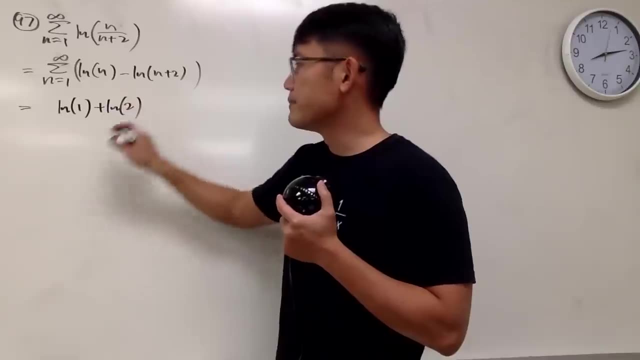 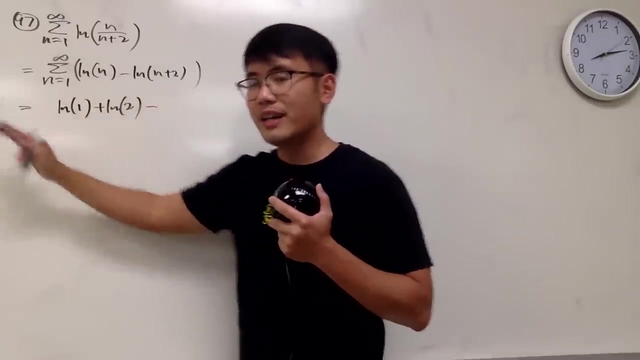 Okay, here we go. This is off by 2.. So we're just plugging the first two numbers. In other words, we get ln 1 plus ln 2, all right, And then you're going to subtract. The first term is going to get cancelled, cancelled, right. 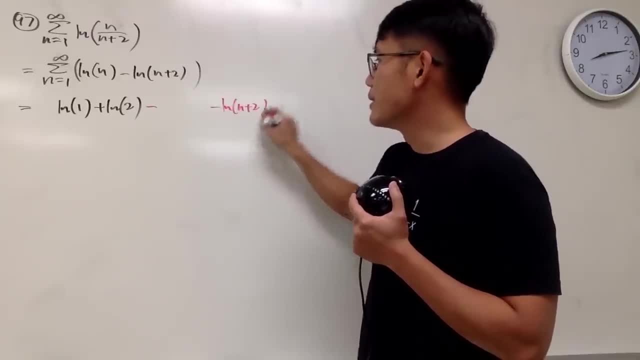 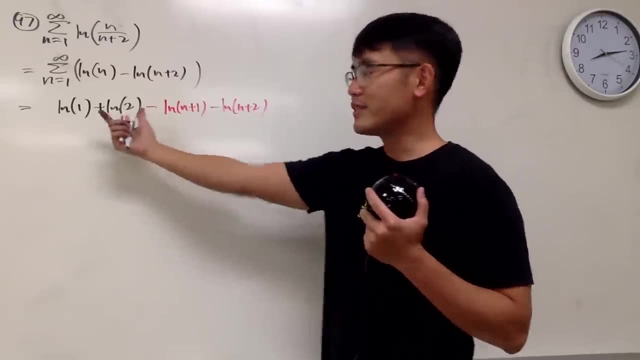 So this is going to be the last term, right: ln of n plus 2.. And then you also have to put on another term before that, So it's ln of n plus 1.. That's it, Okay, seriously, Two things in front, two things in the back. 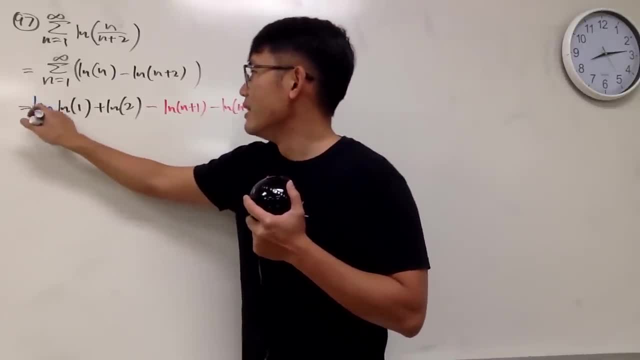 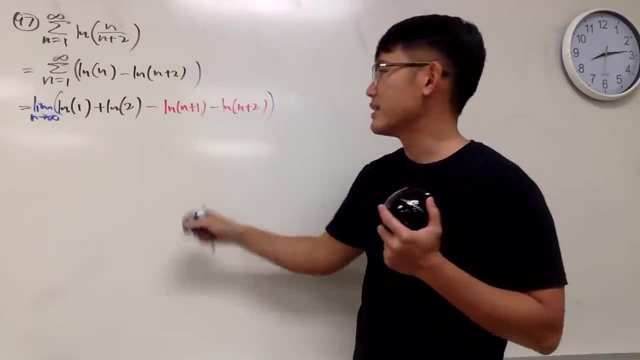 And then you take the limit, And this is the troublesome. The limit as n goes to infinity. of all this, These two guys are innocent, but these two guys aren't. This right here is infinity. So is that? And the worst part is this is minus infinity, minus infinity. 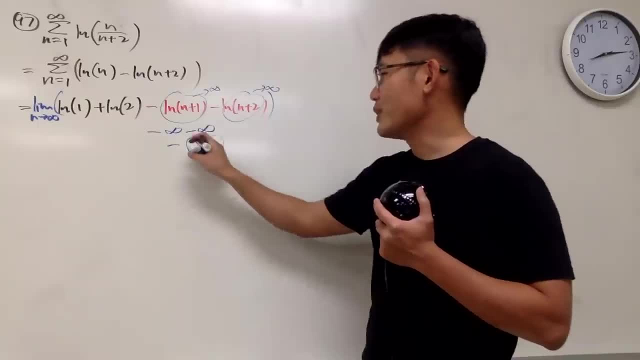 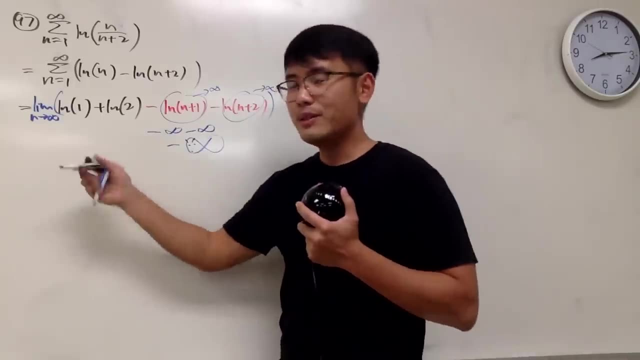 So this is minus a bigger infinity. like that. It's so evil And they also put on like a fish of some kind, right? So this right here actually just like ln 2, because ln 1 is 0. So this right here actually diverges, right. 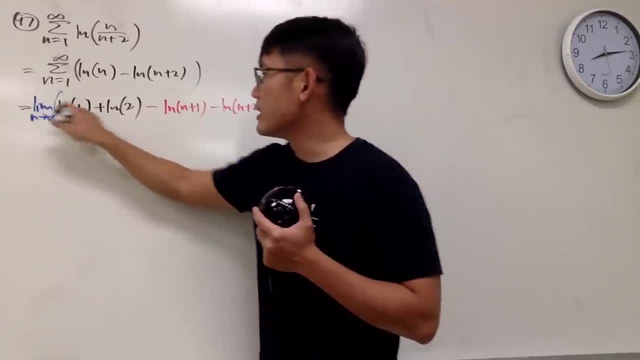 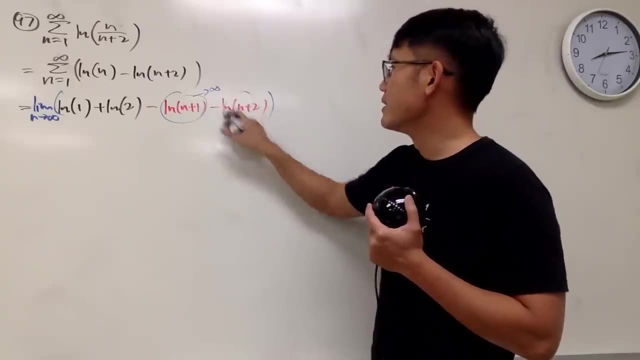 troublesome. the limit as n goes to infinity Of all this. these two guys are innocent, but these two guys aren't. This right here is infinity. so is that? And the worst part is this is minus infinity, minus infinity, so this is minus the bigger. 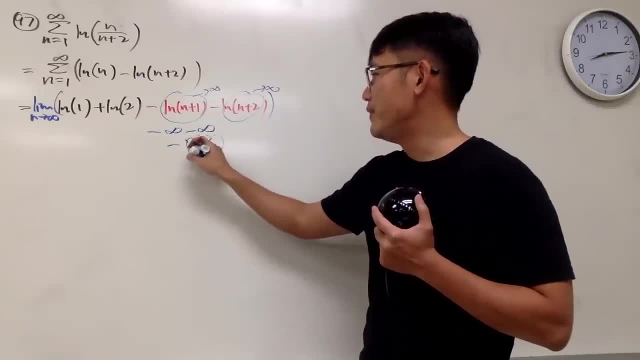 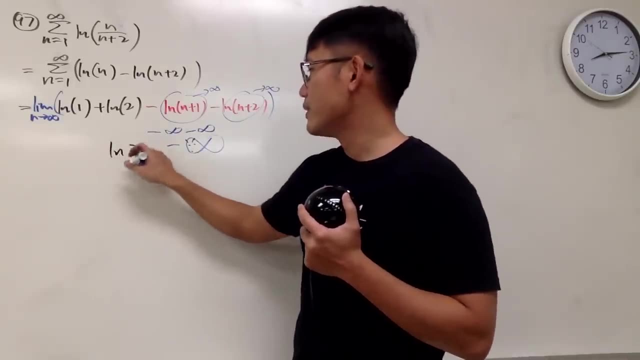 infinity like that. It's like so evil you can also put on like a fish or some kind, all right, So this right here, actually just like ln 2, because ln 1 is 0, so this right here. 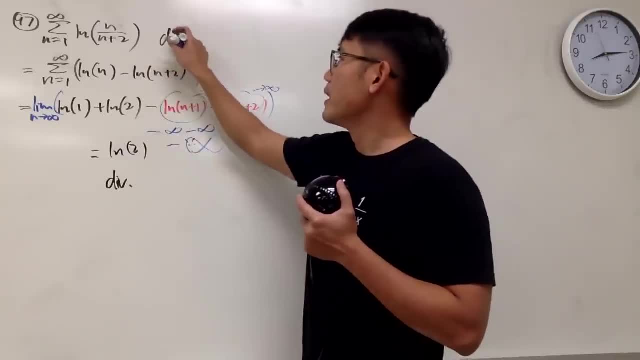 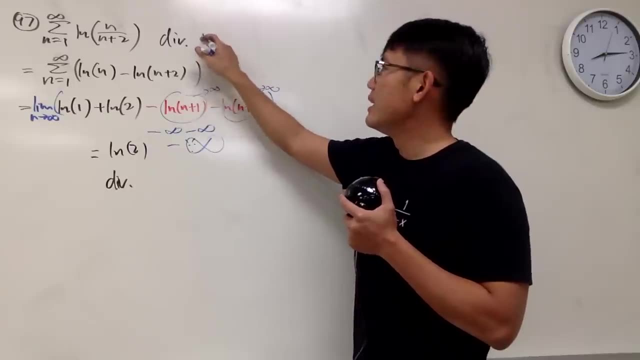 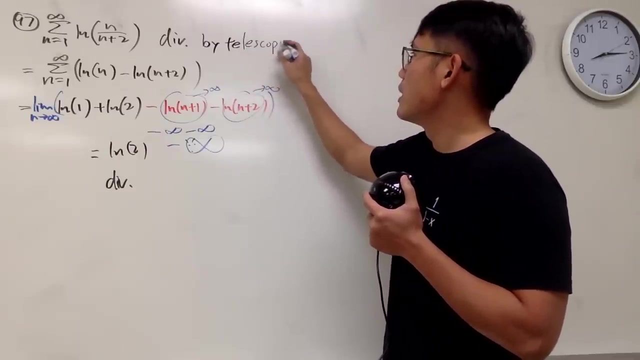 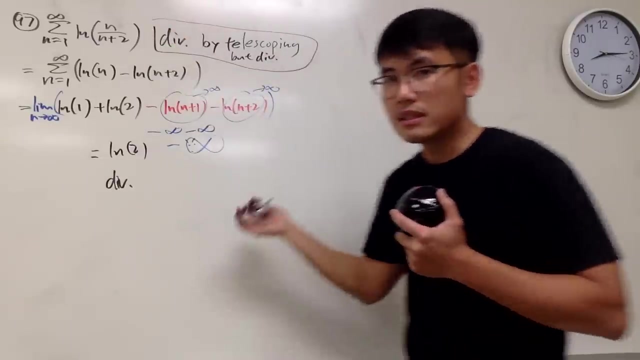 actually diverges right. So diverges Right here I'll just probably say by telescoping series. but it's a diverging telescoping series. Sometimes telescoping might also diverge if the nth term like this part right here. 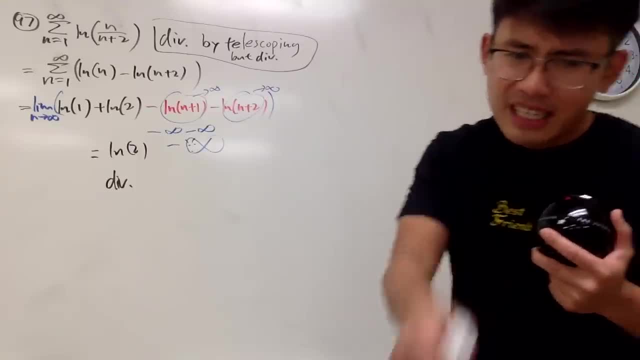 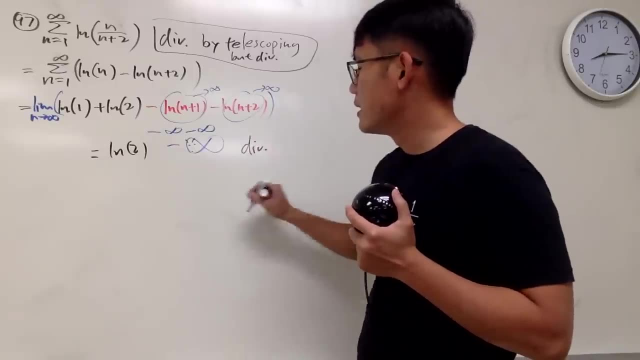 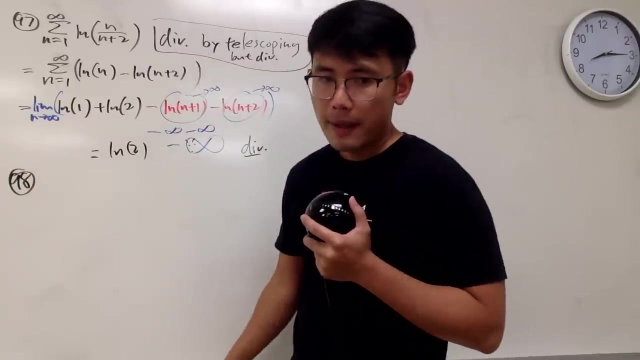 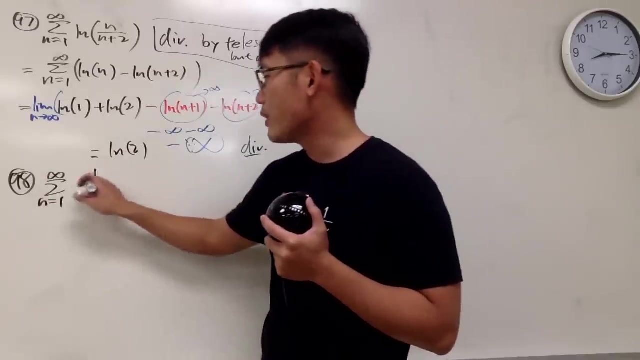 if they don't have, like, a finite limit. it's no good. Number 98,, I'll fit in here. Okay, you guys are with me. Thank you, Number 98.. Here we go, the sum as n goes from 1 to infinity, and here we have 1 over e to the n plus 1,. 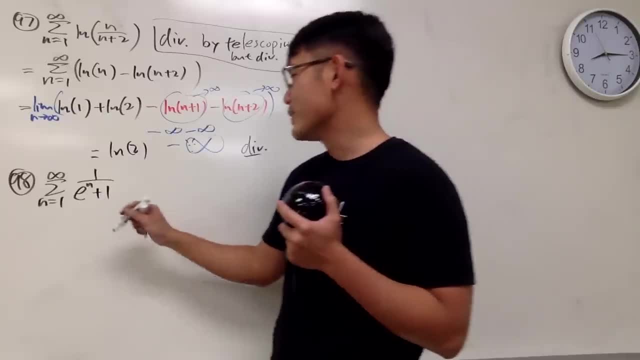 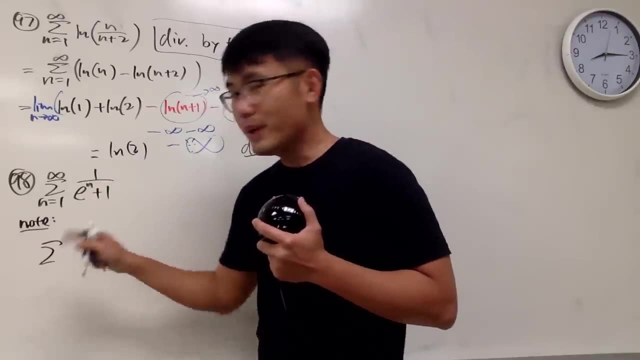 like this Very easy, huh? Yeah, Because we can just right away and say note: Okay, Just minus, just ignore the 1.. And, by the way, if you want to do the integral test for this, go ahead right. 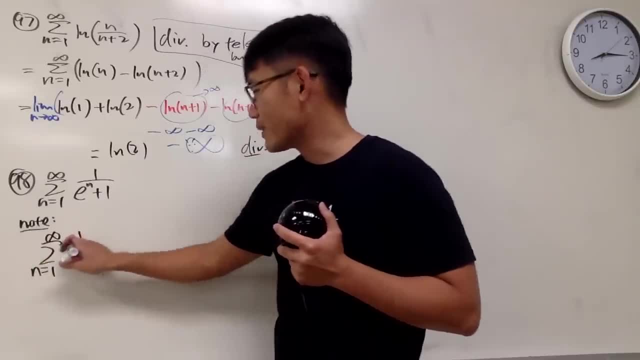 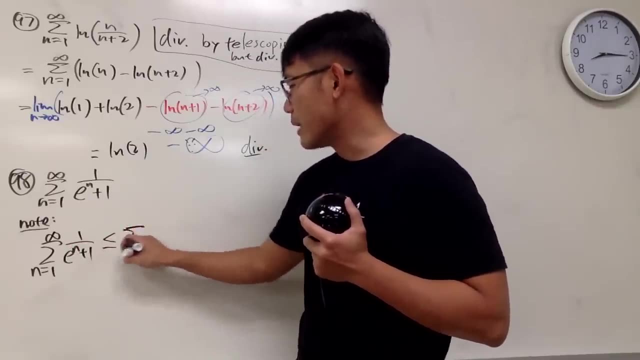 This is integral. it's actually really fun as well. So we have all that. Notice this right here. I will just take away the plus 1, so this is less than or equal to the sum, as n goes from 1 to infinity and we just have 1 over e to the nth power, and 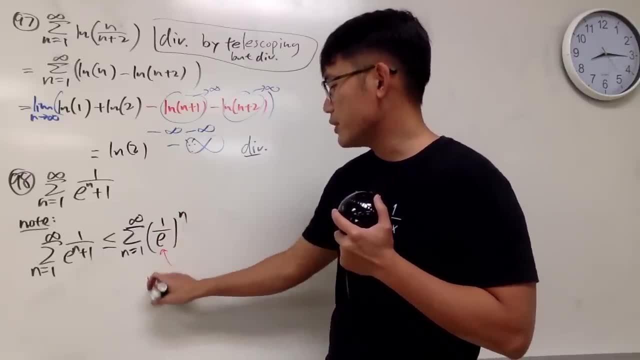 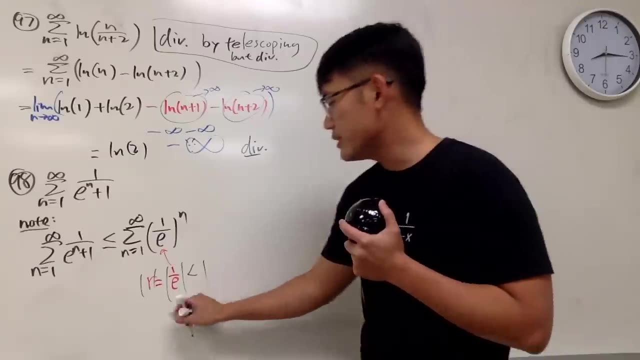 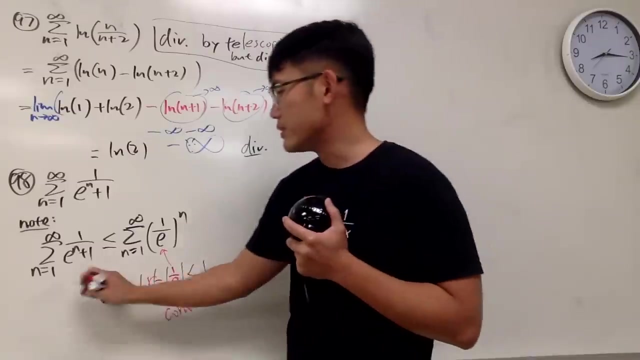 now, let me just put that down as this: This right here is a geometric series which r is equal to 1, over e, Which is less than 1.. And, as you can see, this geometric series actually converges. Therefore, we will come here and say this: also converges. 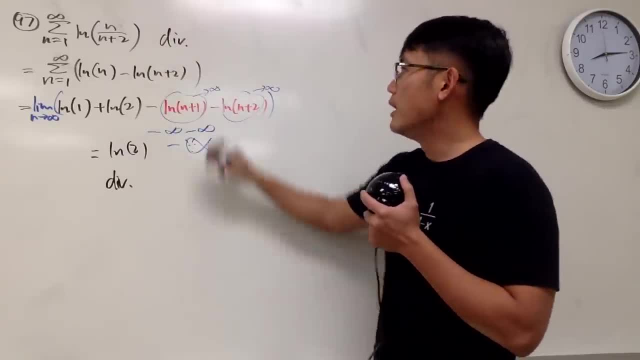 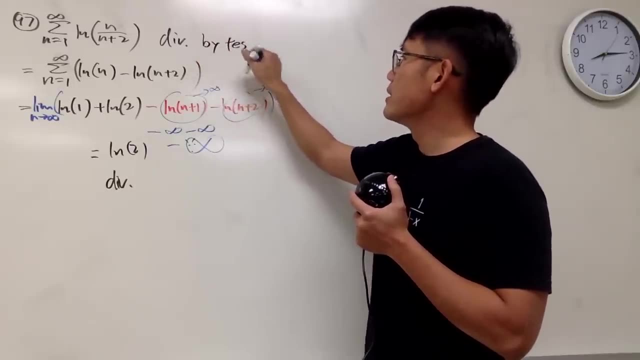 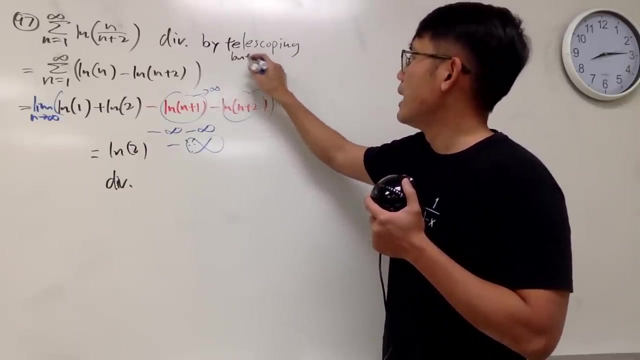 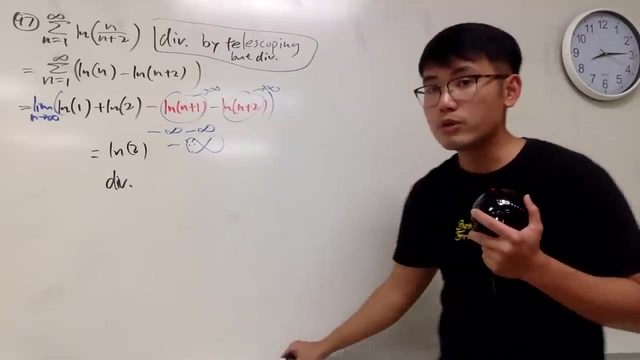 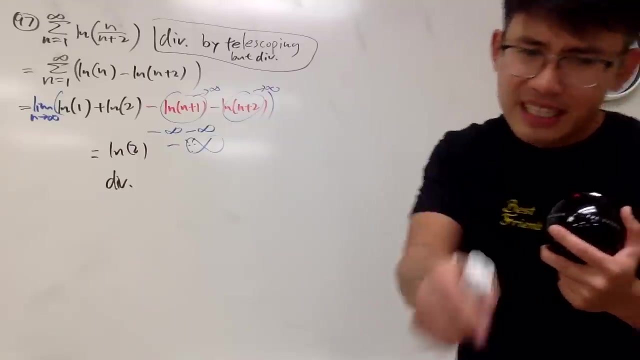 So diverges. Right here I'll just probably say by telescoping series. But it's a diverging telescoping series. Sometimes telescoping might also diverge if the nth term, like this part right here, if they don't have like a finite limit, it's no good. 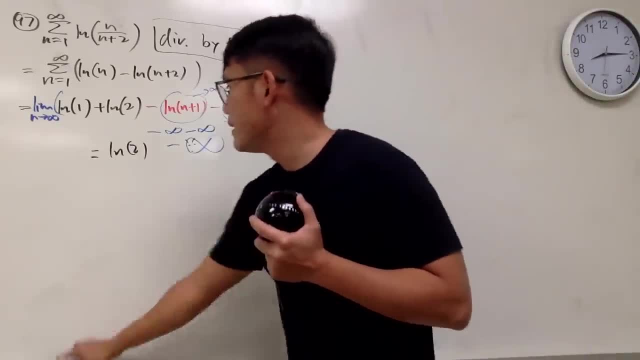 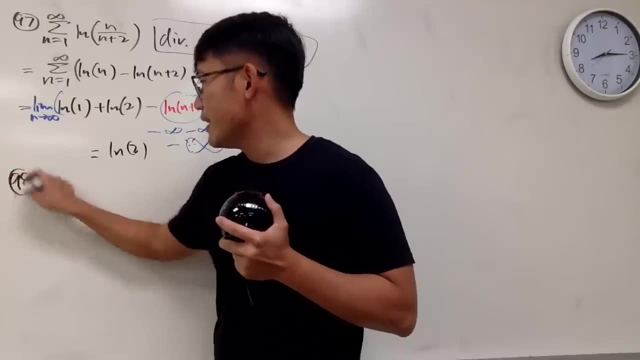 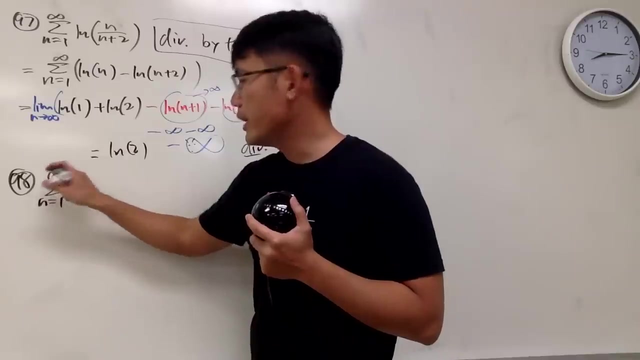 Number 98 will fit in here. Okay, you guys are with me. Thank you, Number 98.. Here we go: The sum as n goes from 1 to infinity. And here we have 1 over e to the n plus 1, like this: 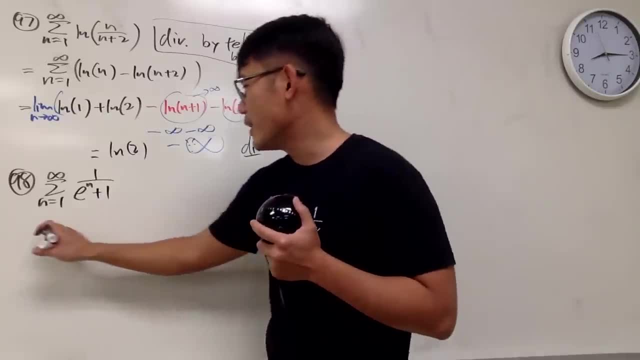 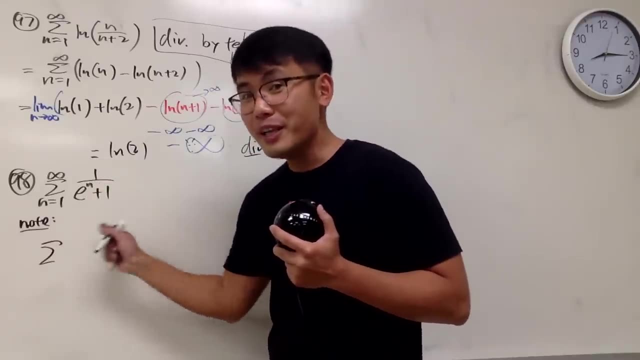 Very easy, huh? Yeah, because we can just right away and say: note: Just minus, just ignore the 1.. And, by the way, if you want to do the integral test for this, go ahead. This integral is actually really fun as well. 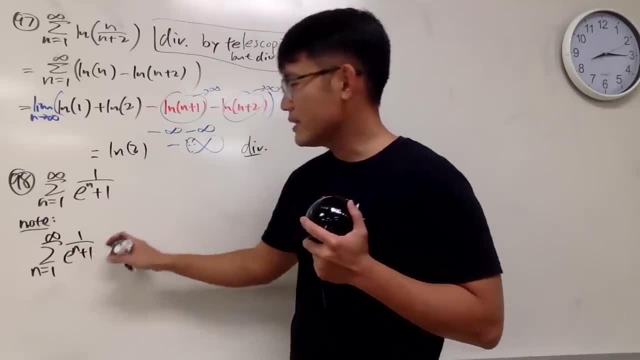 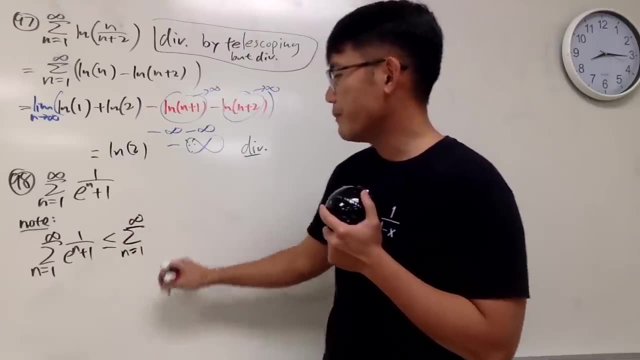 So we have all that. Notice this right here. I will just take away the plus 1.. So this is less than or equal to the sum, as n goes from 1 to infinity And we just have 1 over e to the nth power. 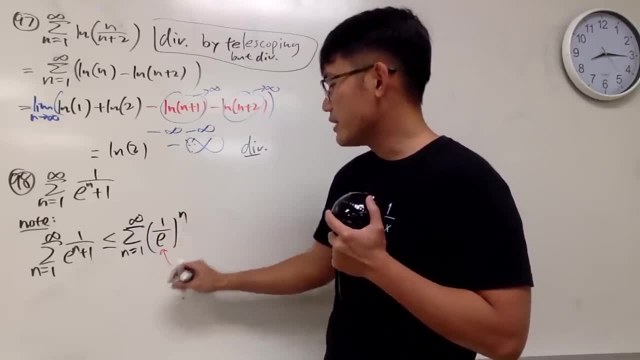 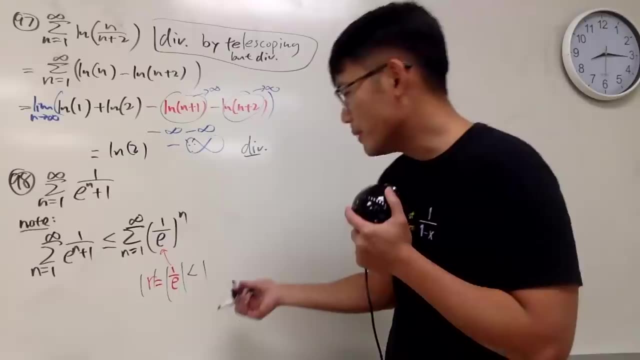 And now let me just put that down as this: This right here is a geometric series which r is equal to 1, over e, which is less than 1.. And, as you can see, this geometric series actually converges. Therefore, we will come here. 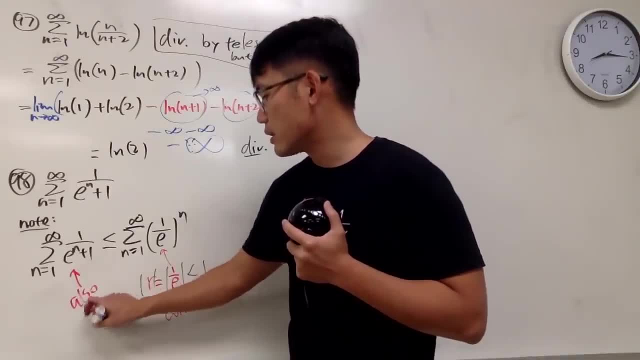 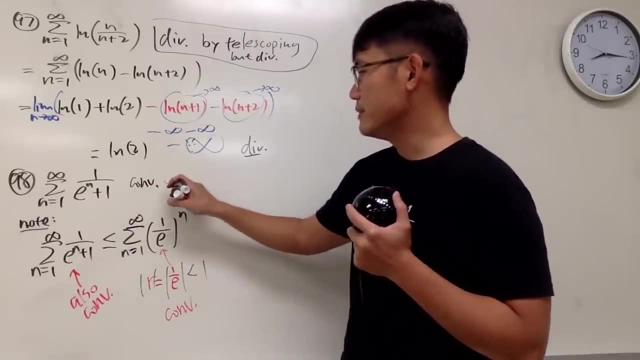 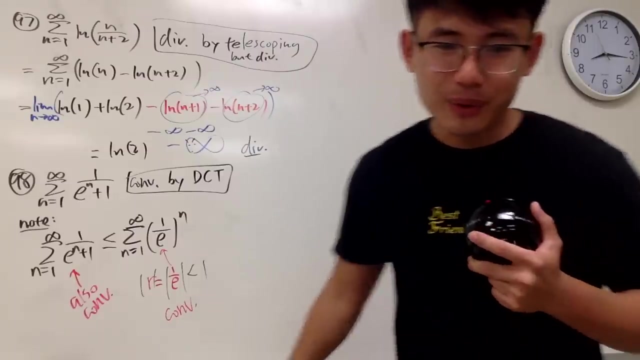 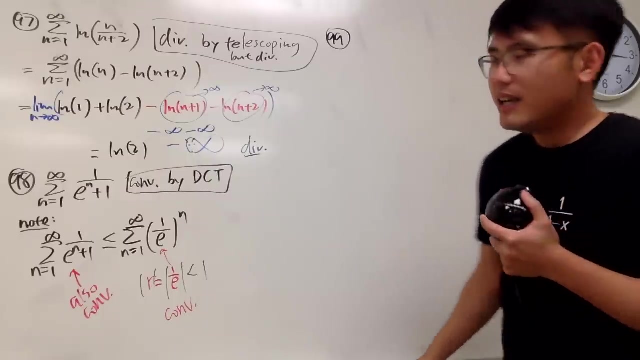 And say this: also converges. So this right here is a convergent, of course. Convergent series by direct comparison test: Alright, so that's it, Very, very cool. Now number 99.. Yes, Alright, just put ln around it. 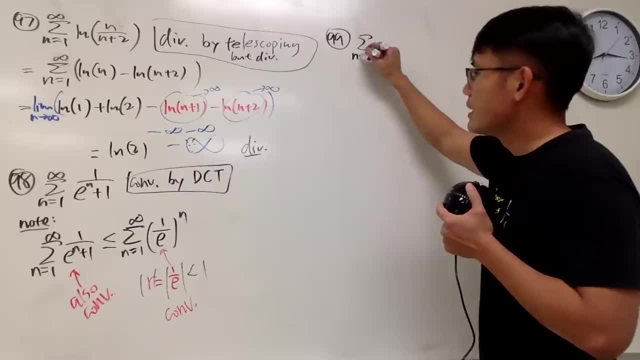 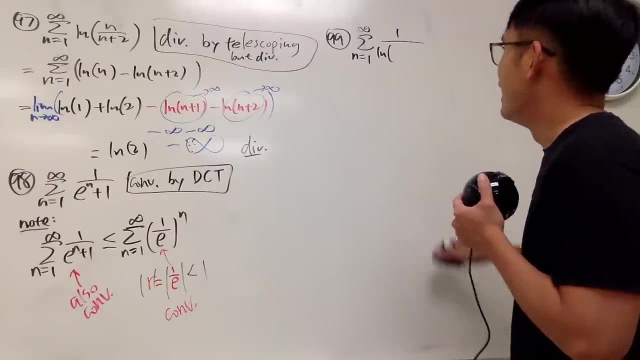 But let's see this one though: The sum as n goes from 1 to infinity, 1 over ln, And just to keep this not so bizarre, I would have to do this as e to the n minus 1.. Like that. 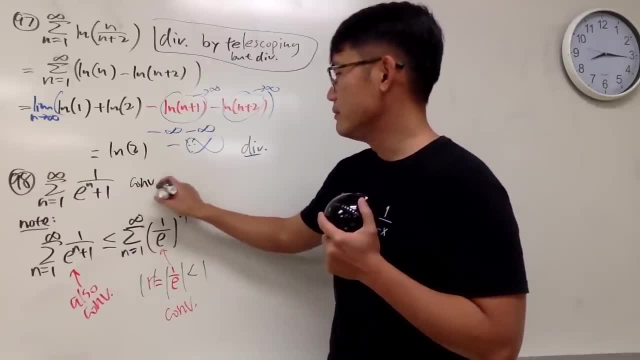 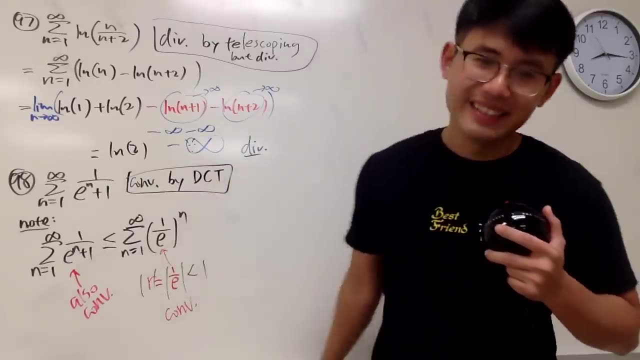 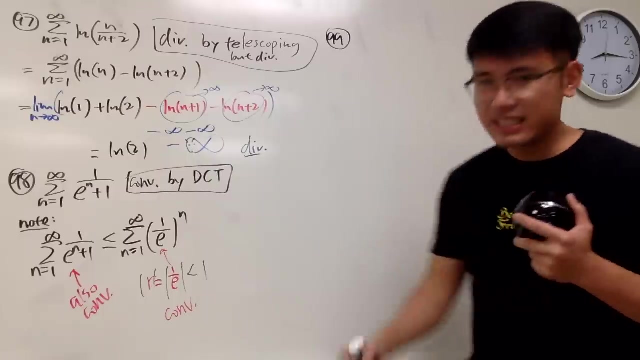 So this right here is a convergent, of course, convergent series by direct comparison test. Okay, So that's it, Very, very cool. Now number 99.. Yes, All right, just put ln around it, But let's see this one though. 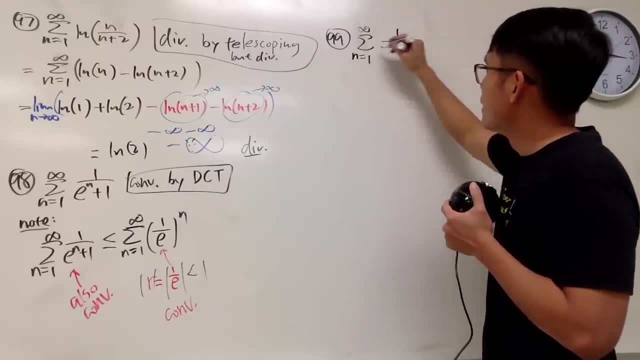 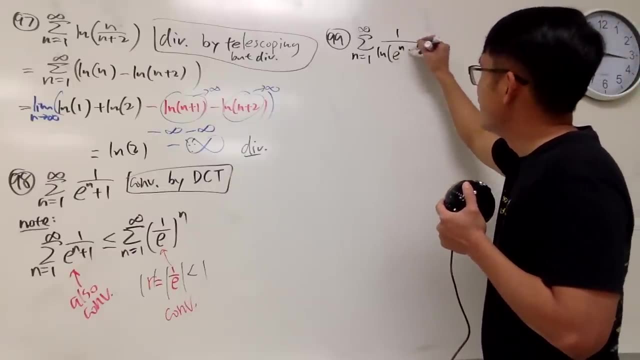 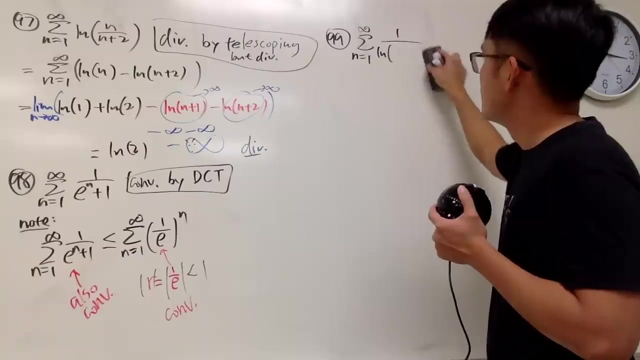 The sum as n goes from 1 to infinity, 1 over ln. and just to keep this not so bizarre, I would have to do this as e to the n minus 1, like that. Okay, Okay, e to the n minus 1.. 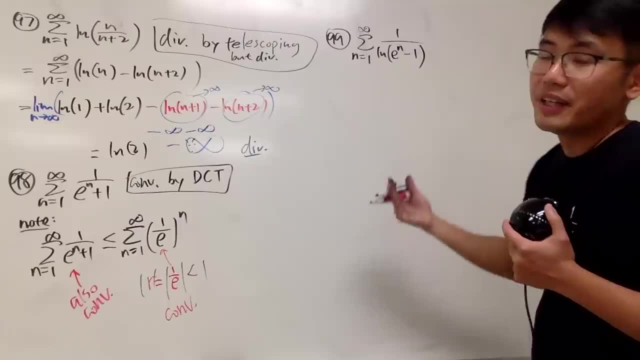 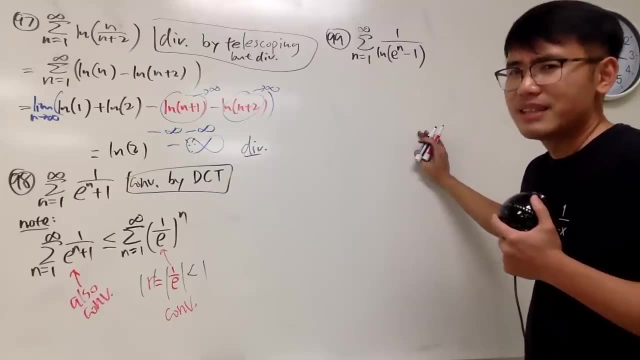 Does it diverge or converge? Earlier, we put in a lot of things in the ln and then, like n to the n, didn't work. So this time, when we have just e to the n, it's not going to work neither. 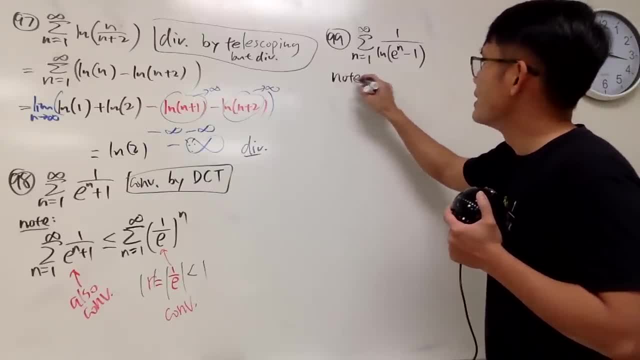 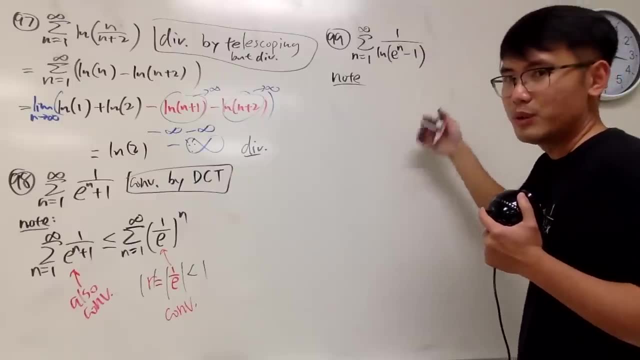 First of all, check this out. Let's make a note. okay, Here we have minus 1 inside and everything like e to the whatever and ln is also increasing function. So check this out, okay. So when we have the sum as n goes from 1 to infinity. 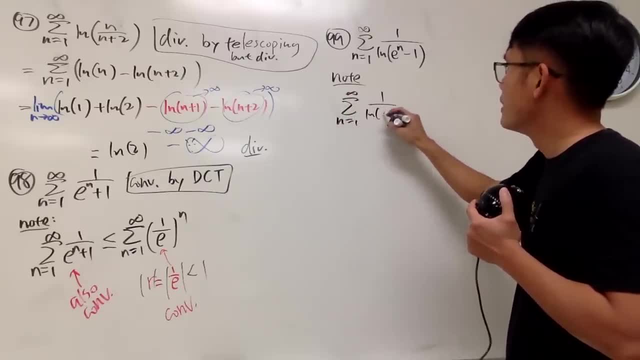 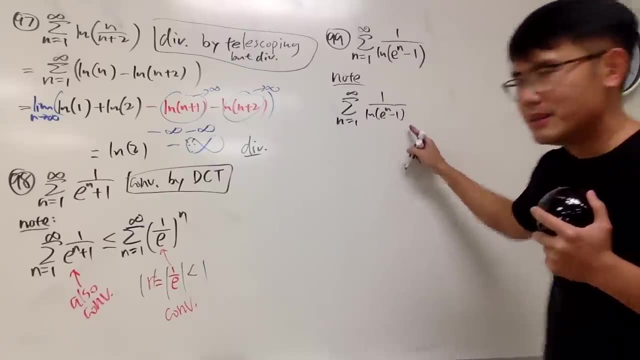 The sum as n goes from 1 to infinity, of 1 over ln e to the n minus 1, I'm going to remove the minus 1.. This time when I remove that, unlike removing a plus 1, when we remove this, let me see: 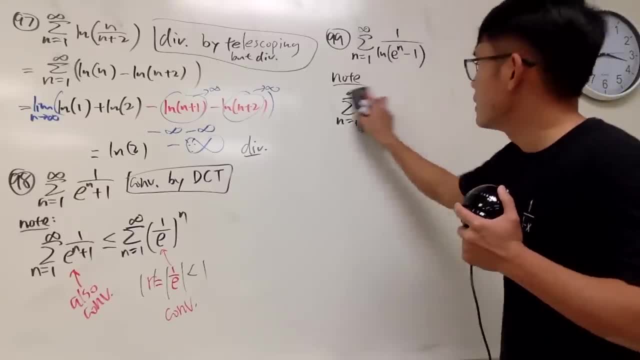 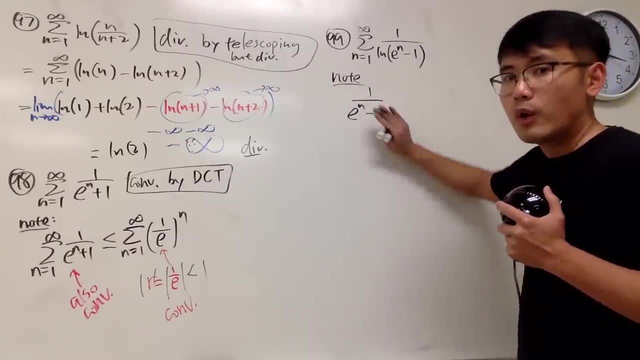 how should I explain that first? Okay, I'll do this for you guys. first Let me just show you guys: 1 over e to the n minus 1.. When we remove the minus 1, the denominator is 1 over e to the n minus 1.. 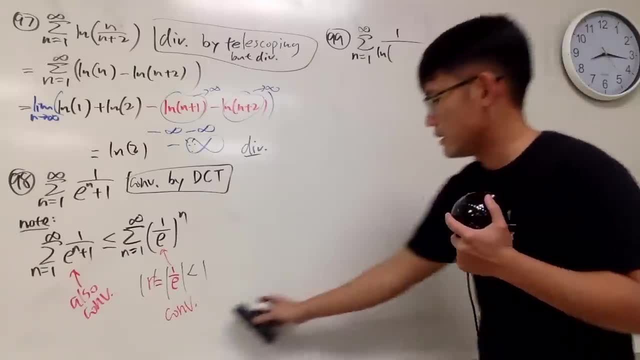 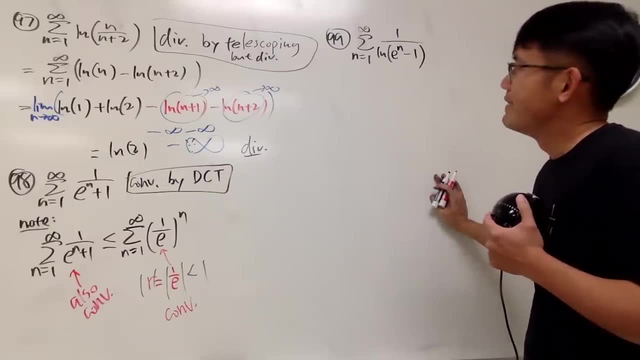 Okay, e to the n minus 1.. Does it diverge or converge? Earlier we put in a lot of things in the ln And then like n to the n. didn't work, So this time, when we have n to the n. 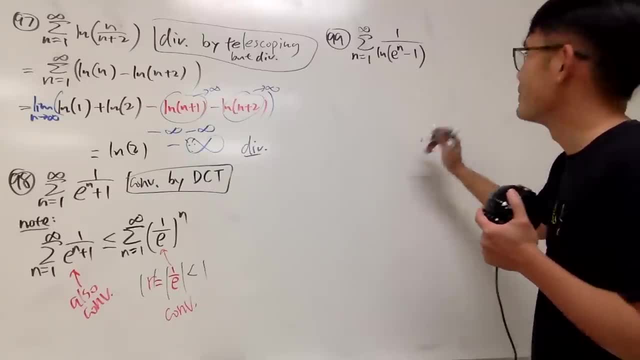 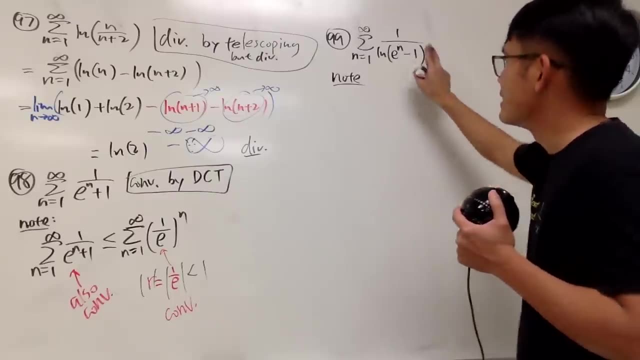 we have just e to the n. It's not going to work neither. First of all, check this out. Let's make a note Here. we have minus 1 inside And everything like e to the whatever, and ln is also increasing function. 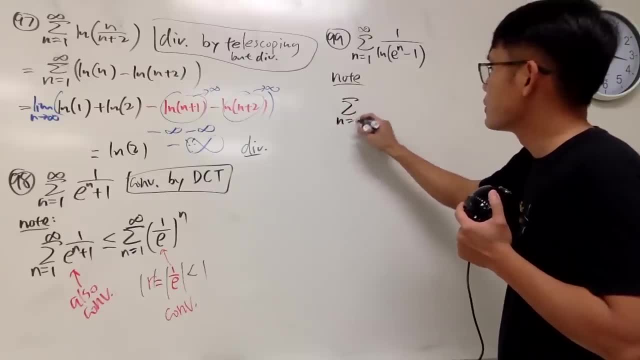 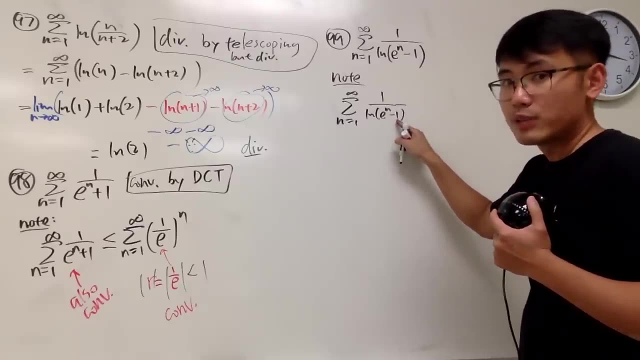 So check this out okay. So when we have the sum, as n goes from 1 to infinity, of 1 over ln, e to the n minus 1, I'm going to remove the minus 1. This time when I remove that, 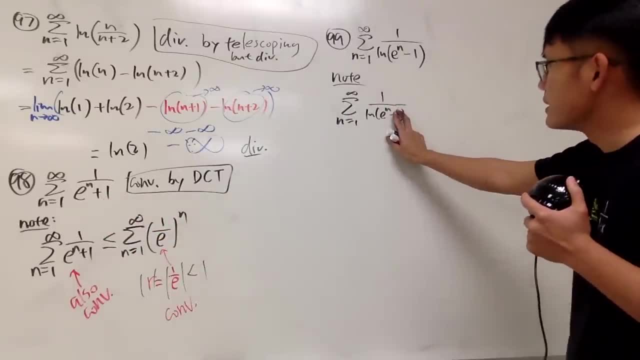 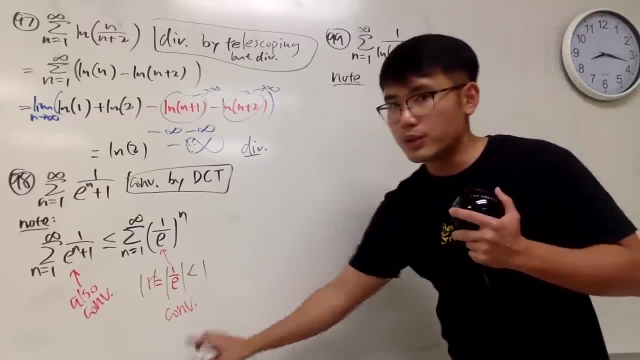 it's like removing a plus 1.. When we remove this, let me see how should I explain that first. Okay, I'll do this for you guys. first Let me just show you guys 1 over e to the n minus 1.. 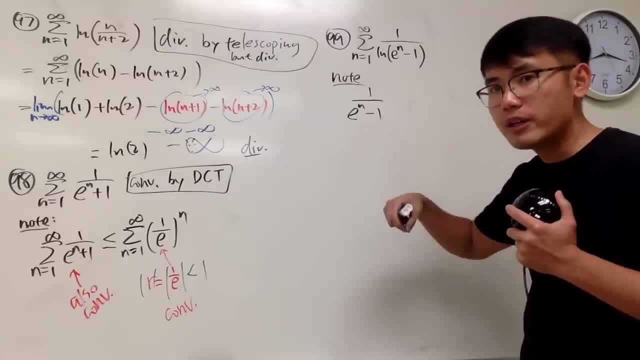 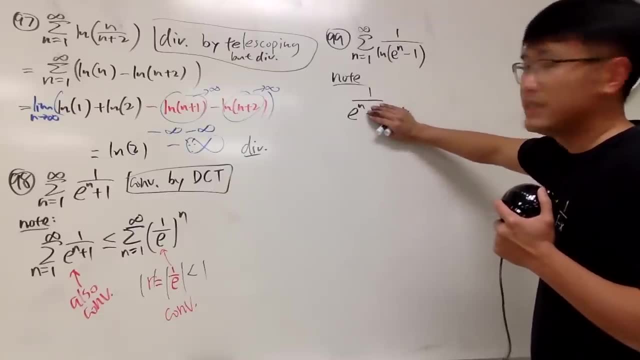 When we remove the minus 1, the denominator is smaller. now I have to remove that. So wait, hold on. When we remove that, this is going to be bigger denominator, so we actually end up with a bigger. this is bigger than 1 over e to the n. 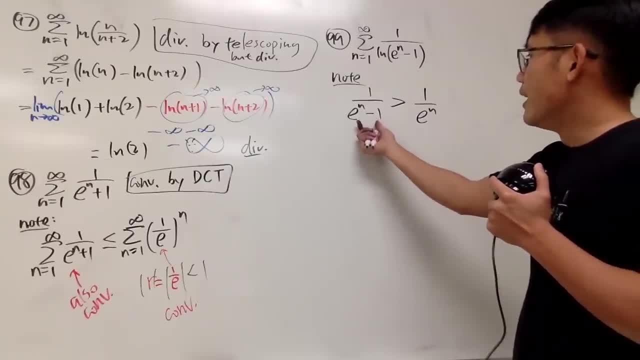 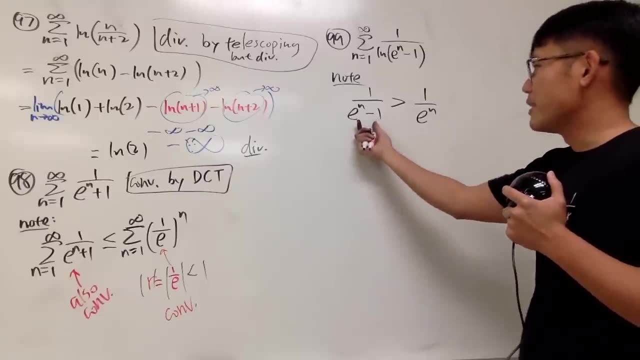 Am I right? Take a look, If you would like. so e to the n is less than e to the negative, 1, right? So this is a smaller denominator, so it's a bigger fraction, you know. So this right here, is true. 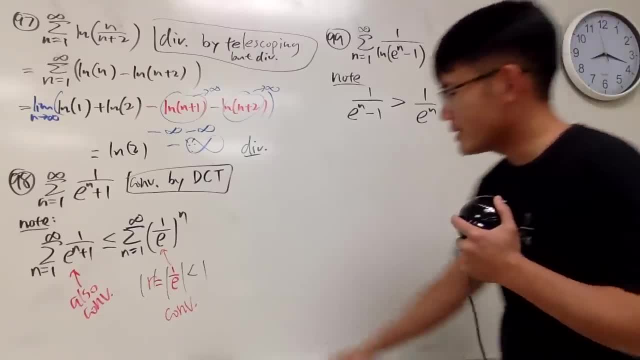 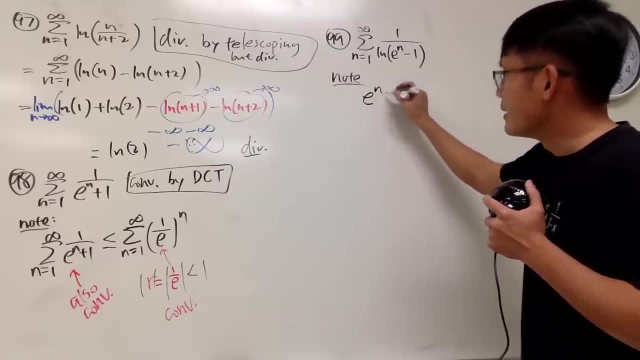 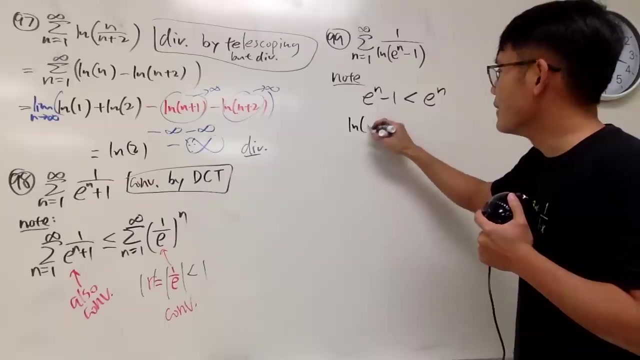 Now, let's do this, Let's do this. So please, okay, okay, okay. e to the n to the n minus 1, is less than e to the n. This is almost like duh. And then you take the natural log: of e to the n minus 1,. 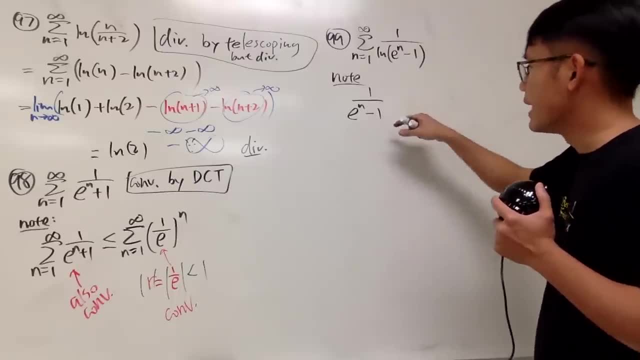 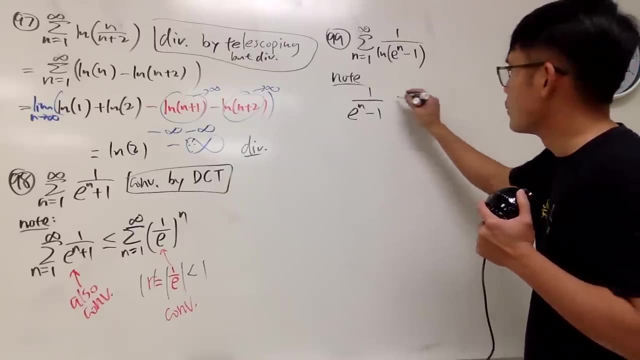 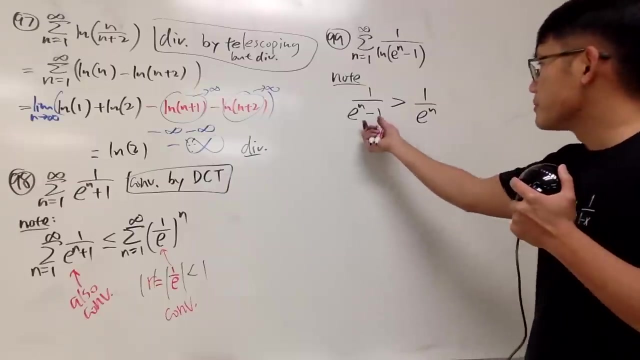 The denominator is smaller now after we remove that. So when we remove that, this is going to be bigger denominator, So we actually end up with a bigger. this is bigger than 1 over e to the n. Am I right? Take a look. 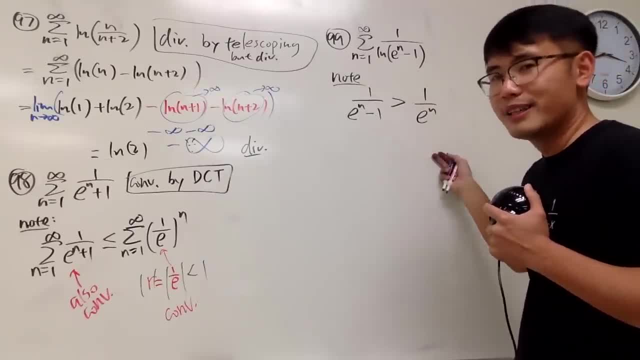 If you would like it's just: e to the n is less than e to the negative 1.. So this is a smaller denominator, so it's a bigger fraction, You know. So this right here is 3 over e to the n minus 1.. 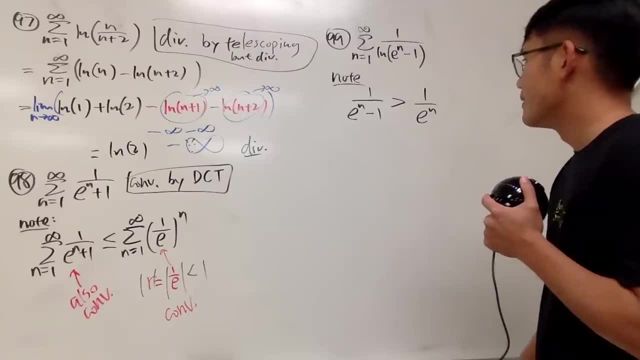 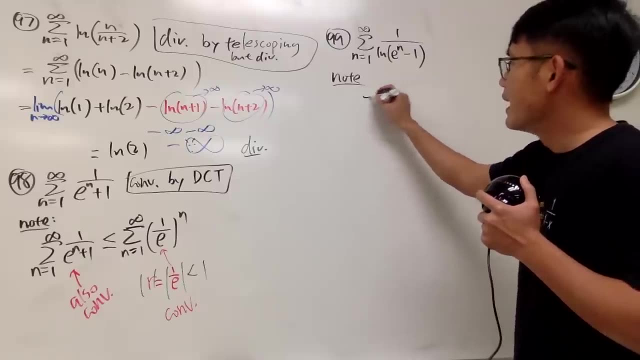 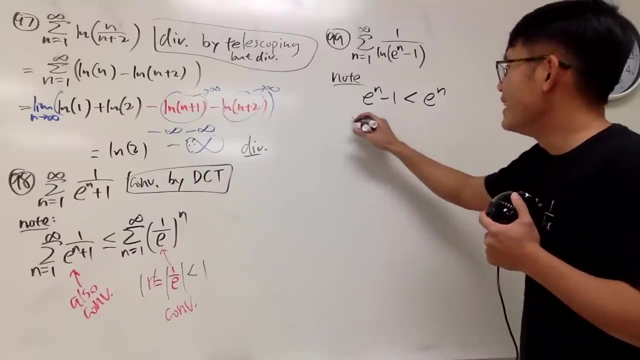 Okay. So this is true. Now you know, let's do this, Let's do this. So please sorry, Okay, Okay, Okay. e to the n minus 1 is less than e to the n. This is almost like duh. 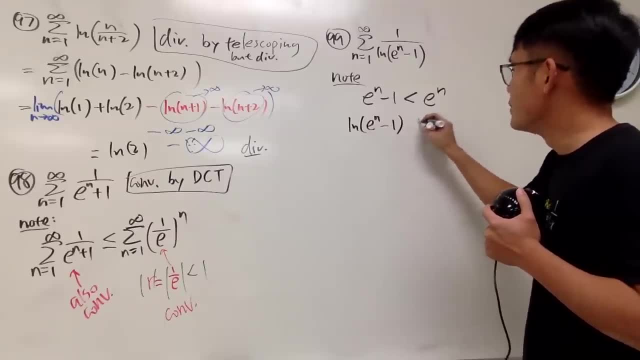 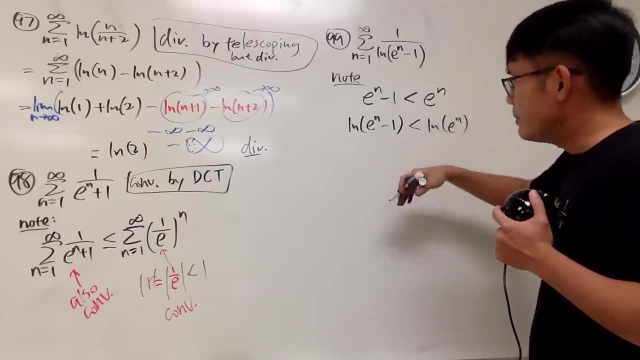 And then you take the natural log of e to the n minus 1, which is still less than natural log of e to the n- That's going to be n later on, right? And then you do the reciprocal and everybody is positive. 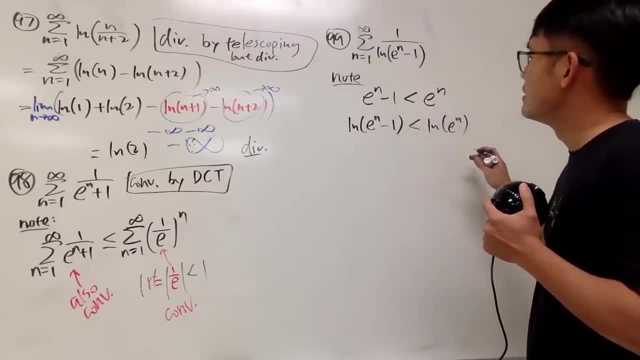 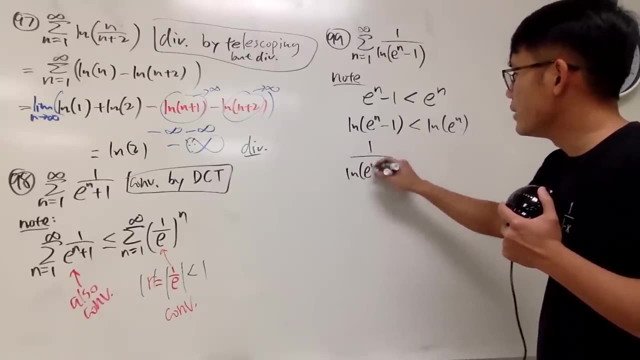 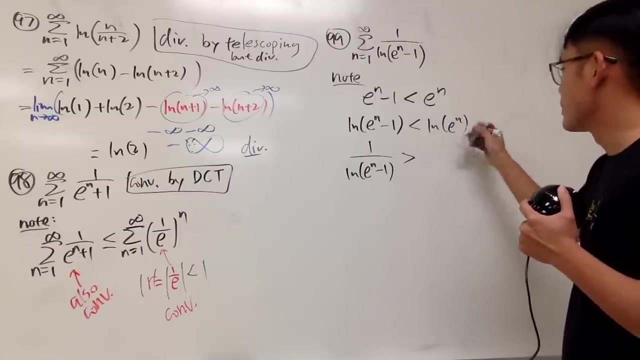 Okay, Let's see. Yeah, Everybody is positive, That's good. So you do the reciprocal. So you get 1 over ln, e to the n minus 1 being greater than 1 over, which is what this right here is just n, which is just 1 over. 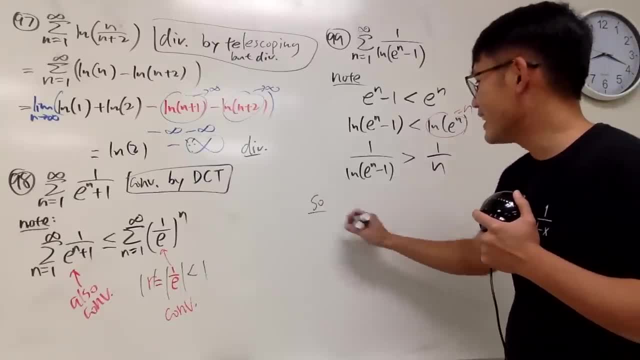 Yay, We just showed that. So we see that the sum as n goes from 1 to infinity, 1 over ln, e to the n minus 1.. Okay, So we have 1 over n, e to the n minus 1.. 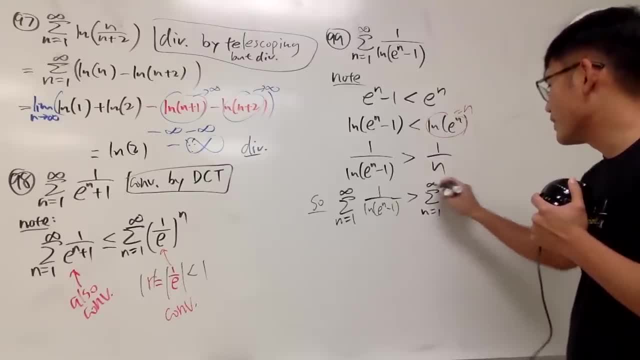 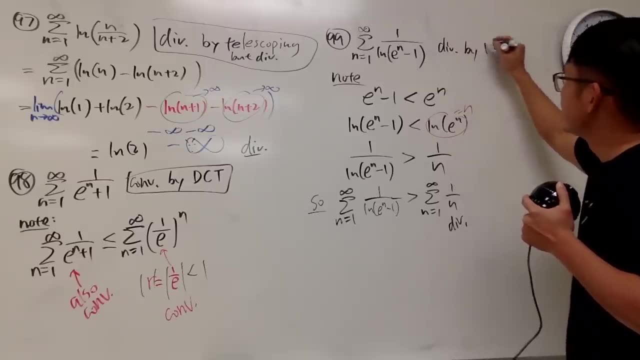 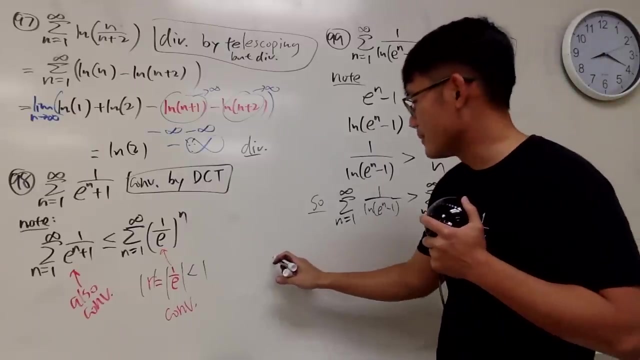 This right here is actually greater than the sum, as n goes from 1 to infinity, 1 over n, And this guy diverges This right here, also diverges right, So diverges by direct comparison test like this: Okay, So that's very, very nice. 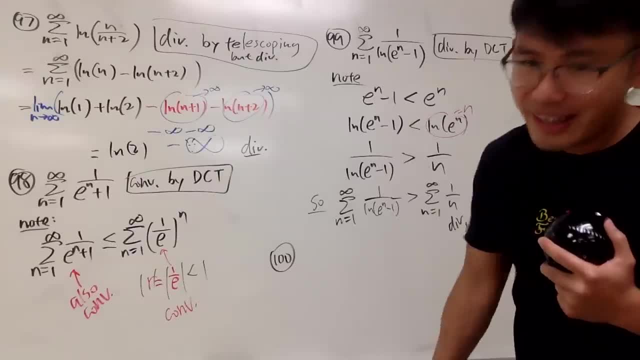 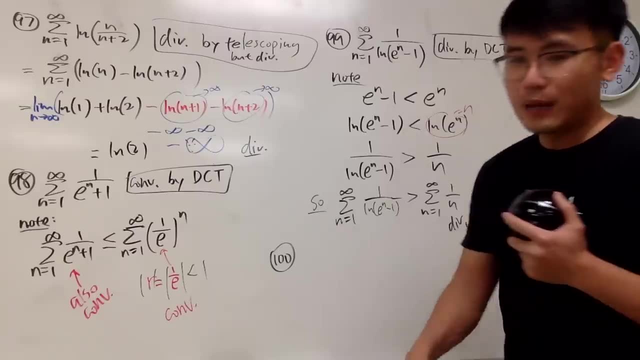 Now number 100, another one that we can actually compute the value for this. So I will write this down for you guys And I really want to change the. I know some of you guys might solve this, but I want to just change this for my own fun. 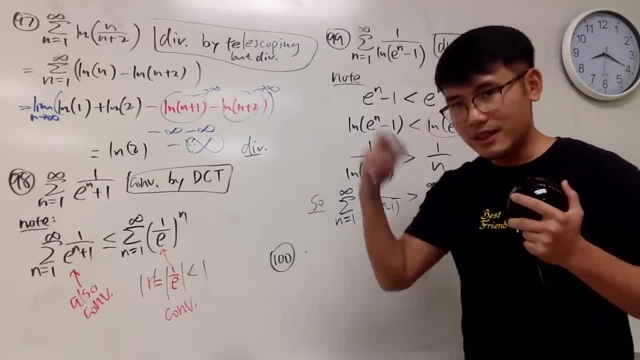 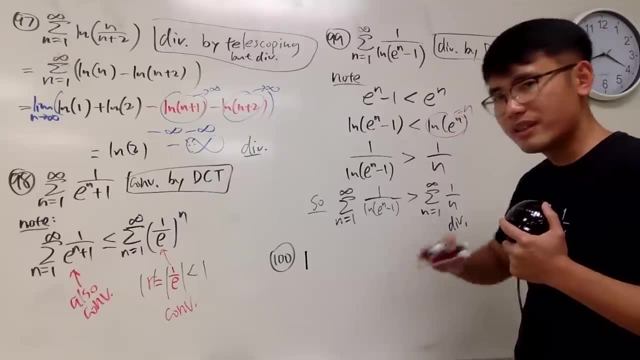 Okay. Okay, How we start it should be how we end. but change it a little bit. If we have 1 plus 1 half plus 1 third plus 1 fourth, that diverges No good. But let me tell you. 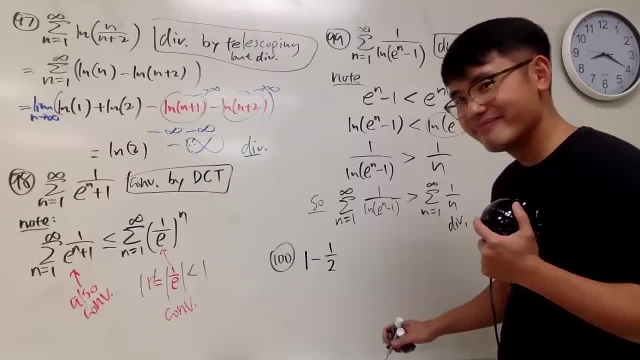 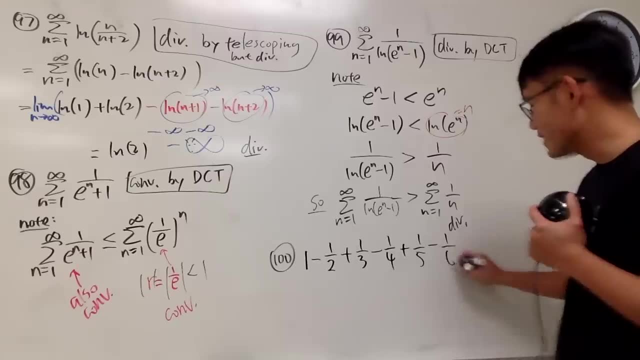 If we have 1 minus 1 over 2, plus 1 over 3, minus 1 over 2.. Okay, Minus 1 over 4, plus 1 over 5, minus 1 over 6, and so on forever. This right here actually converges. 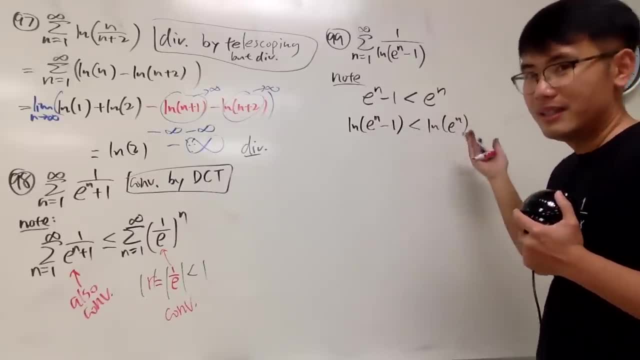 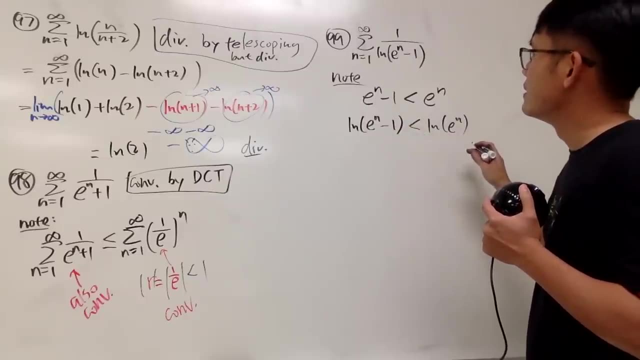 which is still less than natural log of e to the n- That's going to be n later on right. And then you do the reciprocal and everybody is positive. Let's see, Yeah, everybody's positive. That's good. So you do the reciprocal. 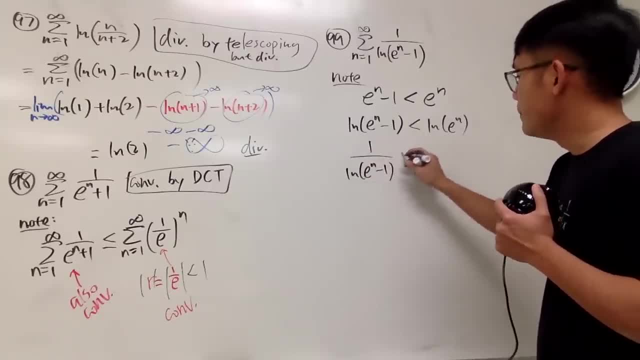 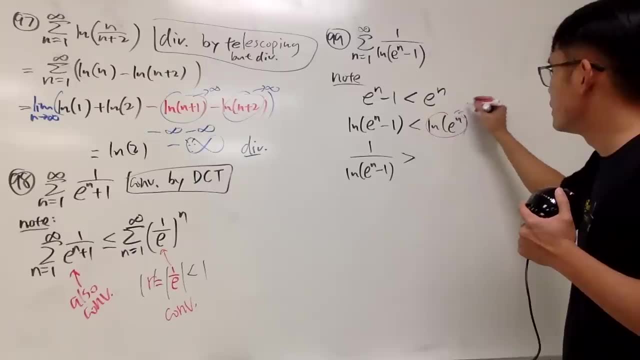 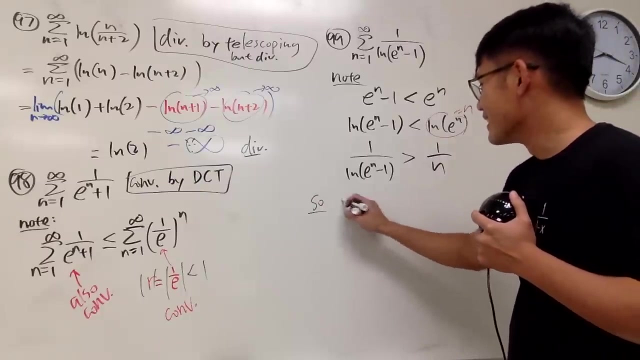 so you get 1 over ln. e to the n minus 1, being greater than 1 over, which is what This right here is just n, Which is just 1 over. Yay, We just showed that. So we see that the sum as n goes from 1 to infinity. 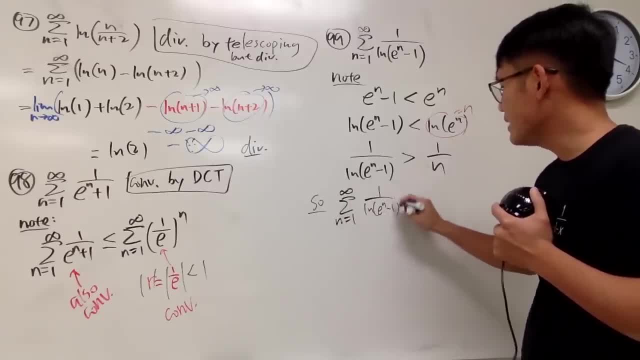 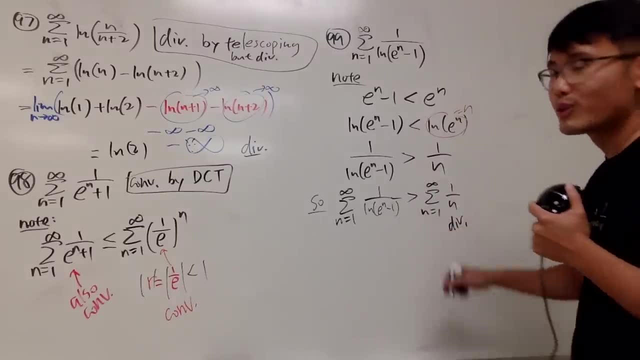 1 over ln, e to the n minus 1.. This right here is actually greater than the sum, as n goes from 1 to infinity, 1 over n, And this guy diverges. This right here also diverges right, So diverges by direct comparison test. 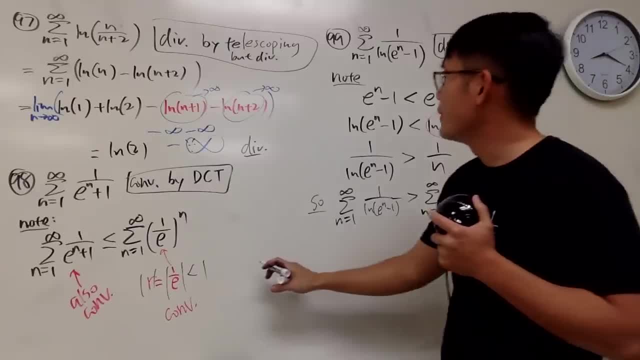 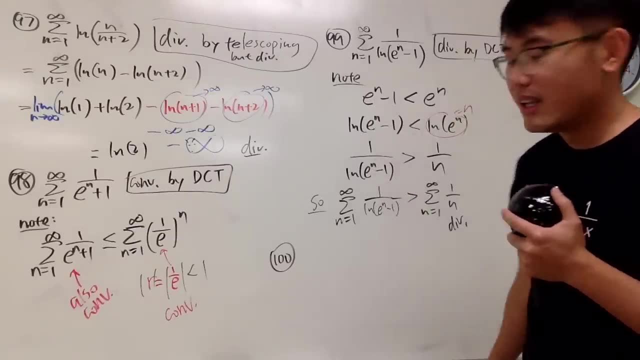 Like this: Okay, So that's very, very nice. Now number 100.. Another one that we can actually compute the value for this. So I will write this down for you guys, And I really want to change the. 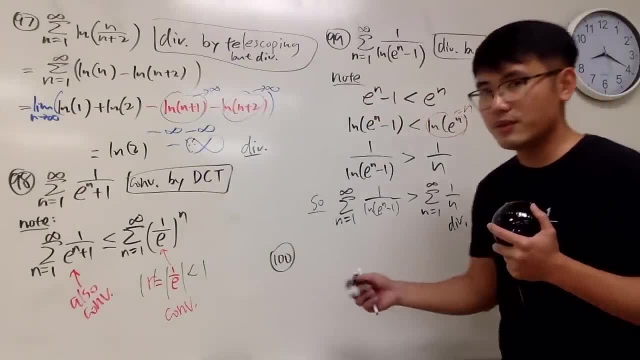 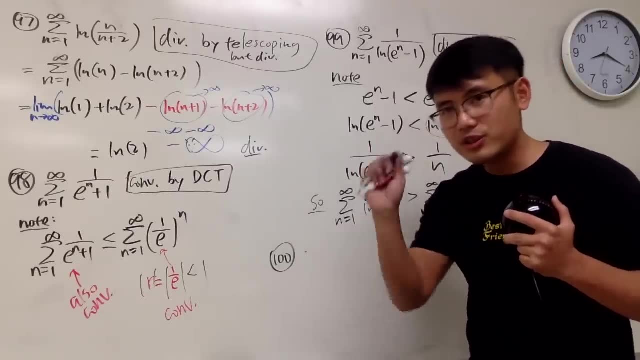 I know some of you guys might solve this, but I want to just change this for my own fun, okay. Okay, How we start it should be how we end, but change it a little bit. If we have 1 plus 1 half plus 1 third plus 1 fourth, 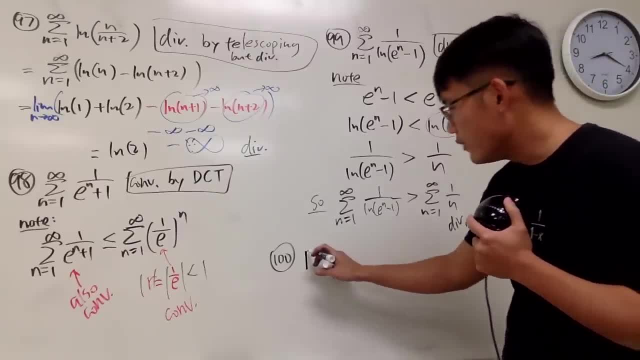 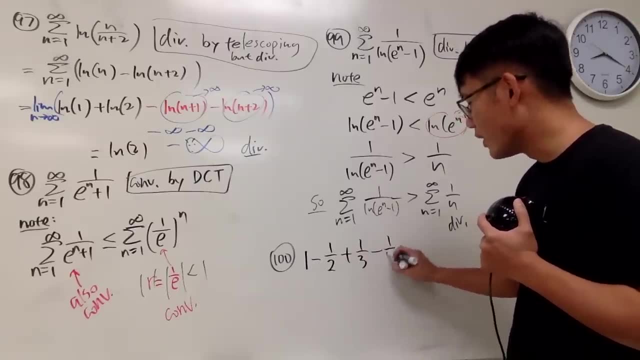 that diverges, No good, But let me tell you, If we have 1 minus 1 over 2, plus 1 over 3, minus 1 over 4,, plus 1 over 5, minus 1 over 6,. 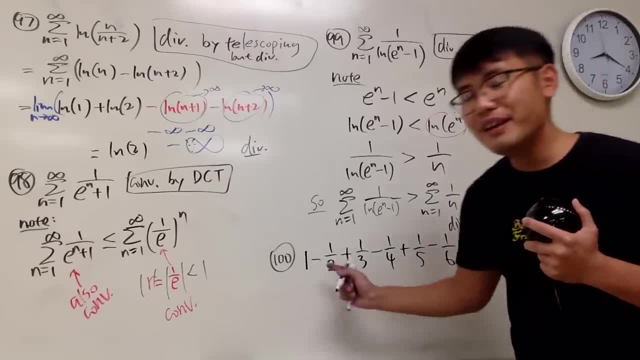 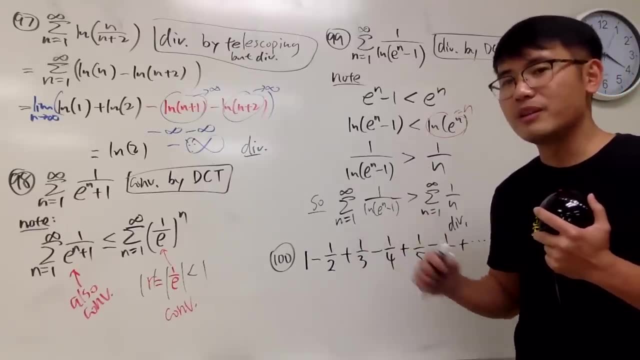 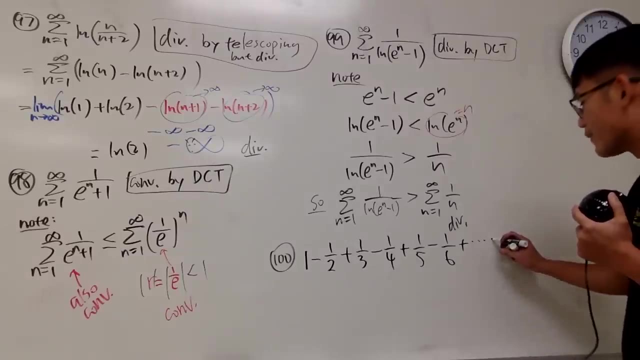 and so on forever. This right here actually converges. This right here, actually, the alternating version of the harmonic series, The alternating version of the harmonic series actually converges, And it converges to Zhuang Ruo, please, 2 ln 2.. 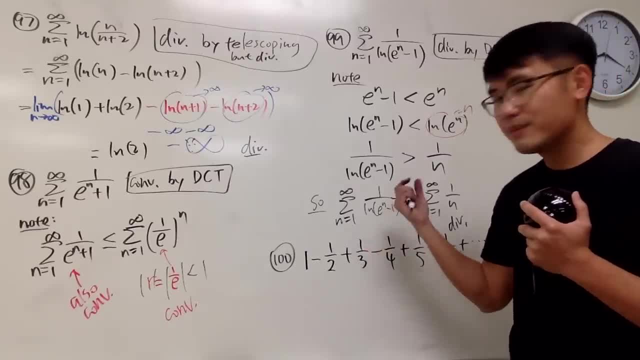 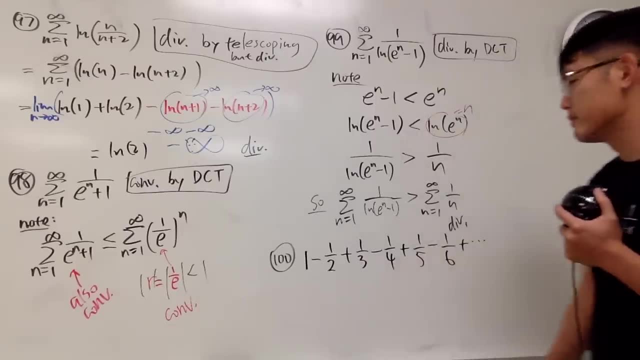 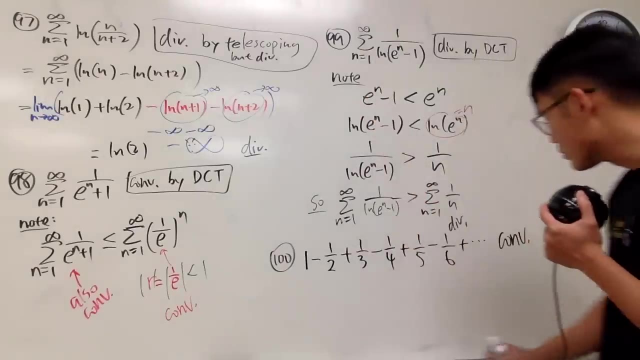 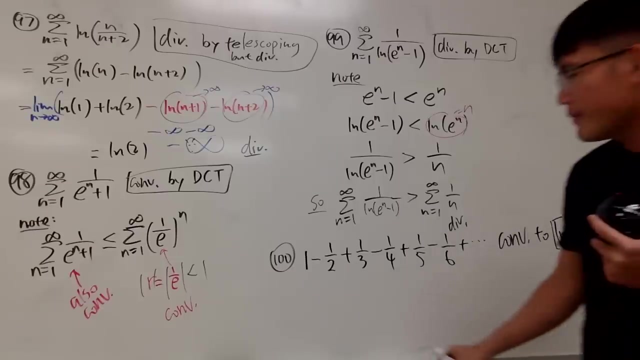 This right here is actually the alternating version of the harmonic series. The alternating version of the harmonic series actually converges, And it converges to Zhuang Ruo, please, To Ln2.. How did we do it? Well, you have to utilize the best friend right. 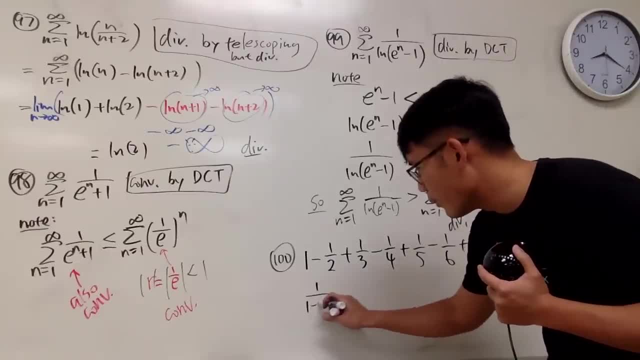 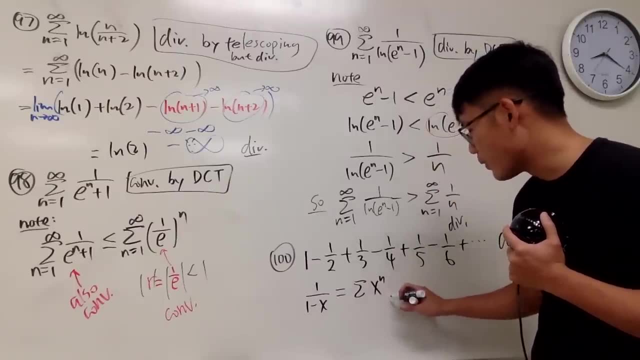 So let me just show you guys this real quick: 1 over 1 minus x, which is the best friend. This right here is the sum as x to the nth power. like this right For n goes from 0 to infinity. 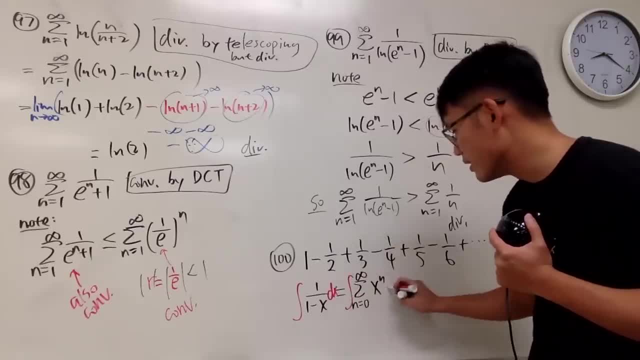 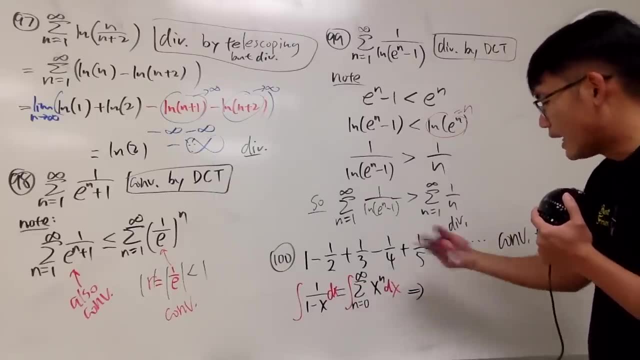 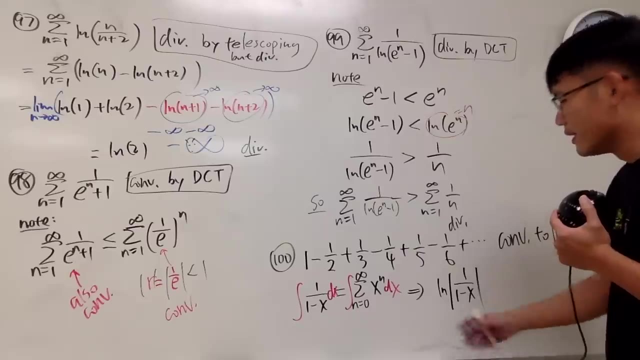 And we are going to integrate our best friend this time And remember, Remember when we integrate our best friend, this is what we get Here. we get Ln of the best friend, right, Ln of our best friend Absolutely technically, but it doesn't really matter that much. 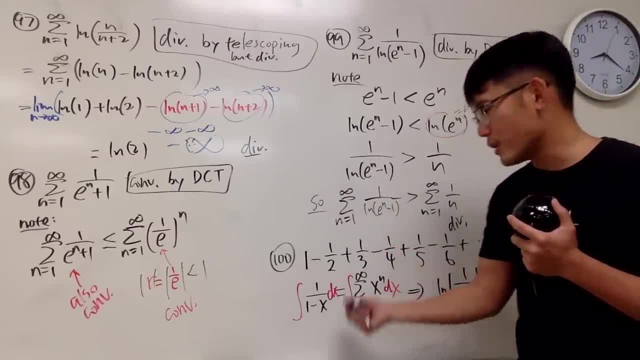 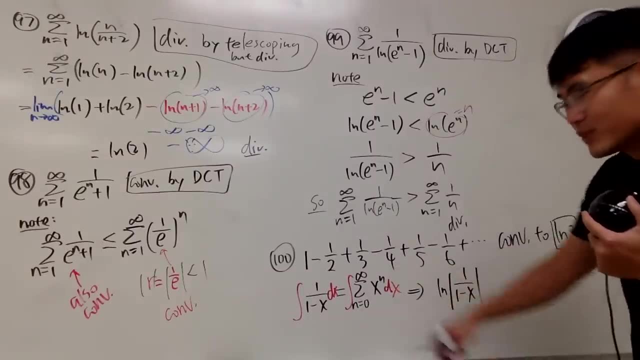 If you guys want to see how to do this, you can check out my other video which I integrated 100 best friend. right, I integrated the best friend 100 times, so I'm not going to do that And in fact this is the last question I did over there, so check that out. 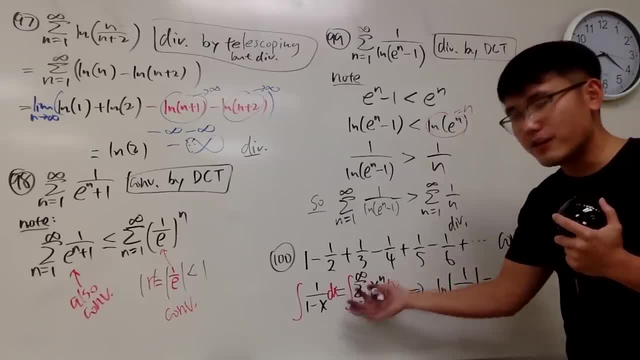 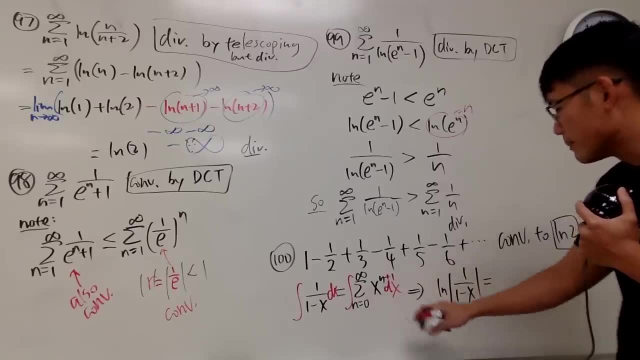 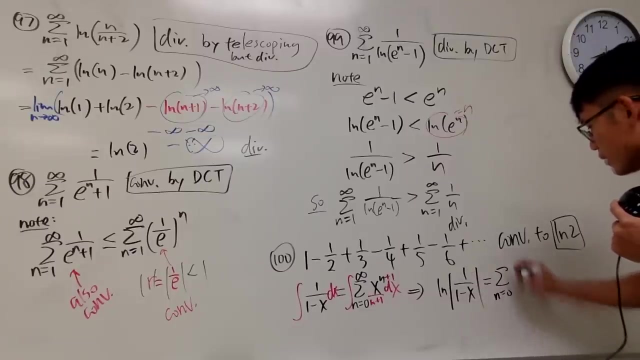 Anyway this: right here you have the constant of the integration, but that's equal to 0. You add 1 to the power and divide it by the power, So you have n plus 1.. So we have this being the sum as n going from 0 to infinity. 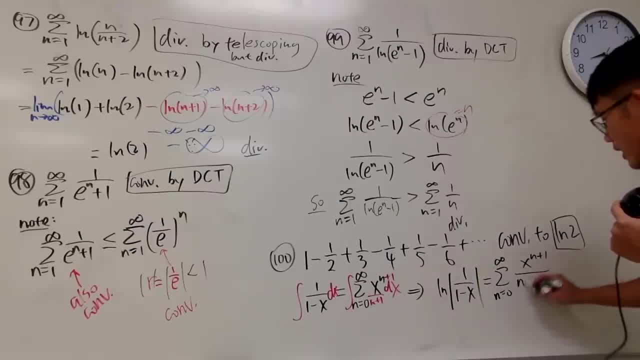 And we have x to the n plus 1, power over n plus 1, like this. And now you might be wondering: how in the world did we end up with this? Well, magic, No, just kidding. Well, technically it's like magic, right. 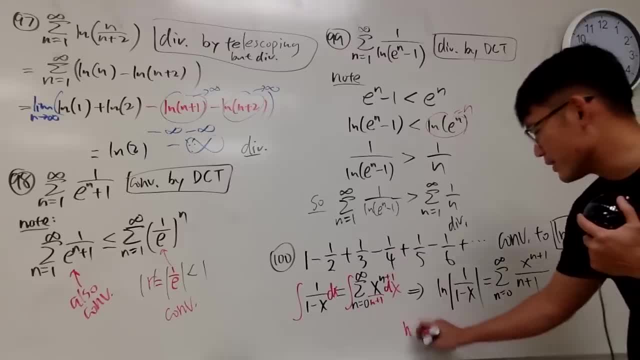 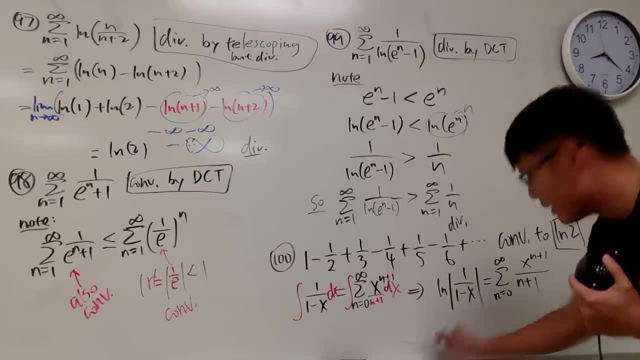 You just let. I will just give you guys a hint, right, I'm just going to give you guys a hint, because I'm kind of running out of space. No, I'm going to finish it. All right, I'm doing blue. 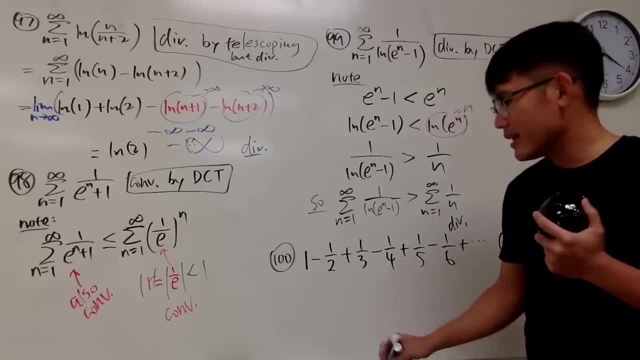 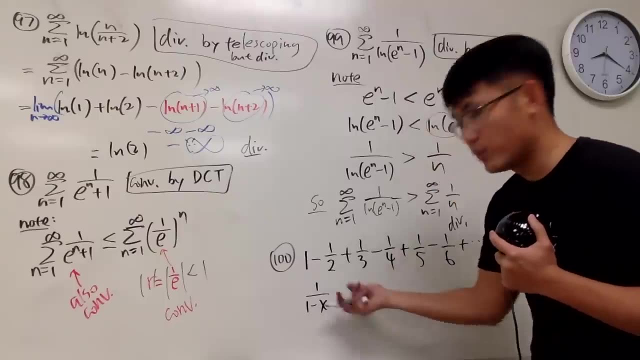 How do we do it? Well, you have to utilize the best friend right. So let me just show you guys this real quick: 1 over 1 minus x, which is the best friend. This right here is the sum as x to the nth power. 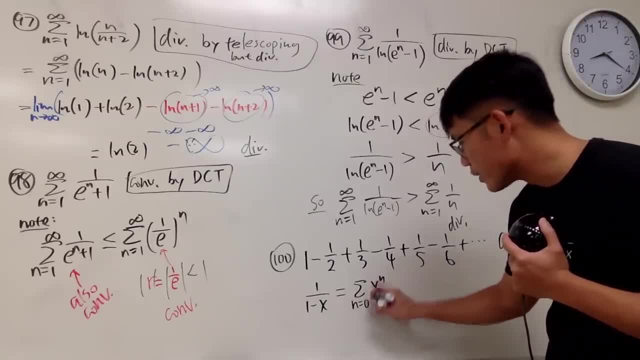 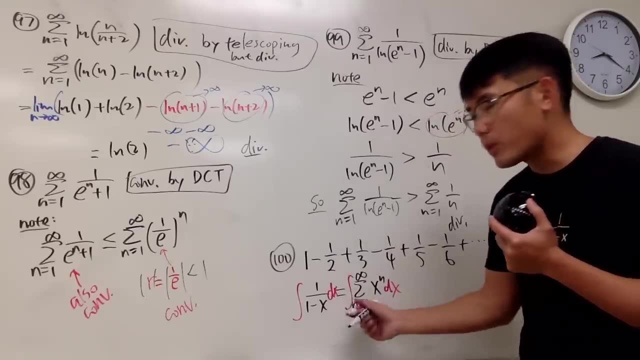 like this right For n goes from 0 to infinity And we are going to integrate our best friend this time, And remember when we integrate our best friend. this is what we get Here. we get ln of the best friend right. 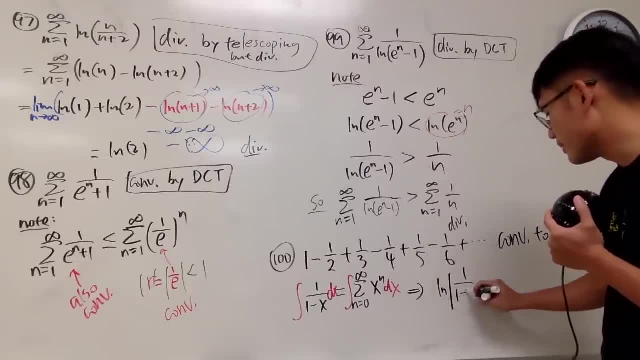 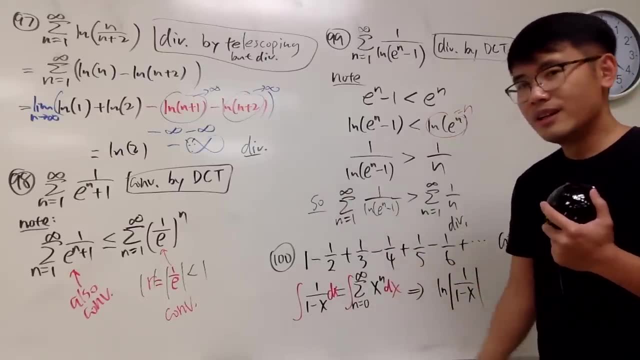 ln of our best friend, But it's not technically, but it doesn't really matter that much. If you guys want to see how to do this, you can check out my other video, which I integrated 100 best friends. right, I integrated the best friend 100 times, so I'm not going to do that. 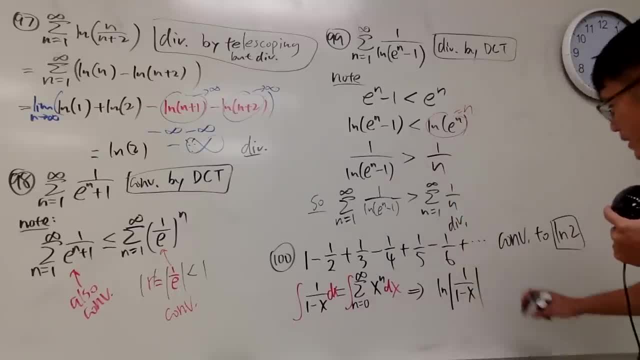 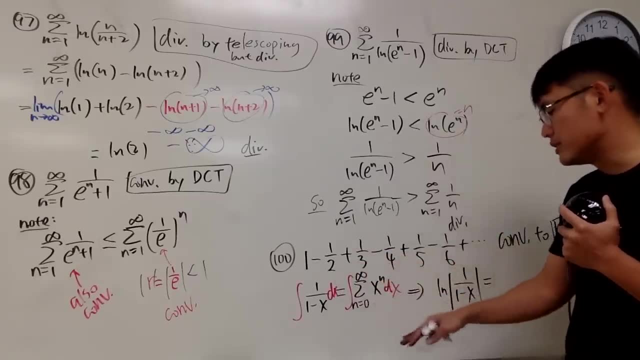 And in fact this is the last question I did over there, so check that out. Anyway, this right here you have the constant of the integration, but that's equal to 0. You add 1 to the power and divide it by the power. 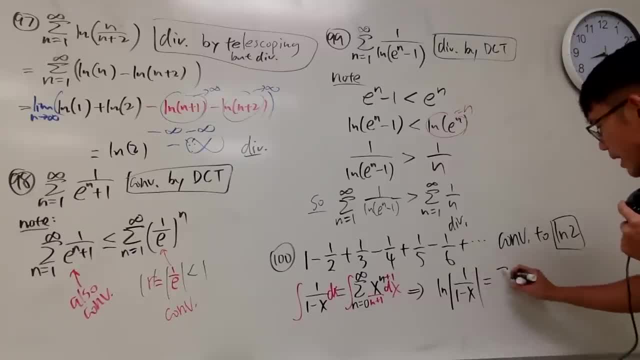 so you have n plus 1.. So we have this being the sum as n going from 0 to infinity, and we have x to the n plus 1 power over n plus 1, like this. And now you might be wondering: how in the world did we end up with this? 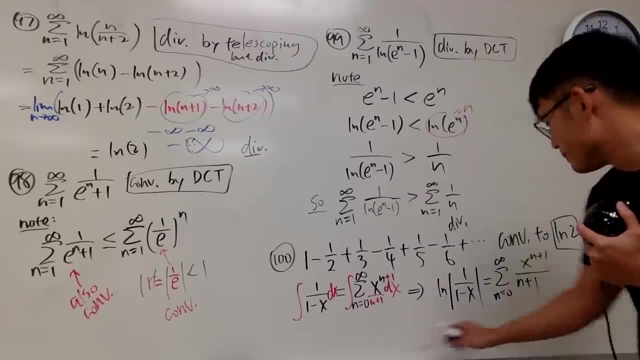 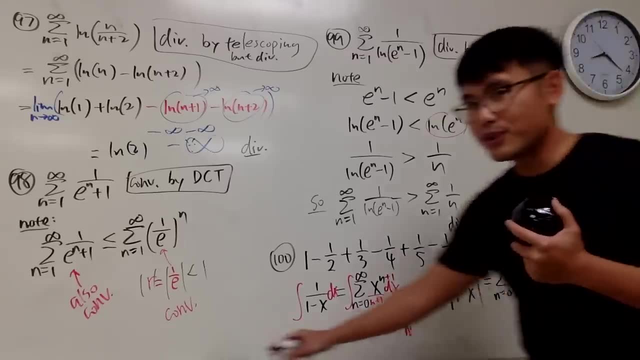 Well, magic, No, just kidding. Well, technically it's like magic, right, You just let, I will just give you guys a hint, right, I'm just going to give you guys a hint because I'm kind of running out of space. 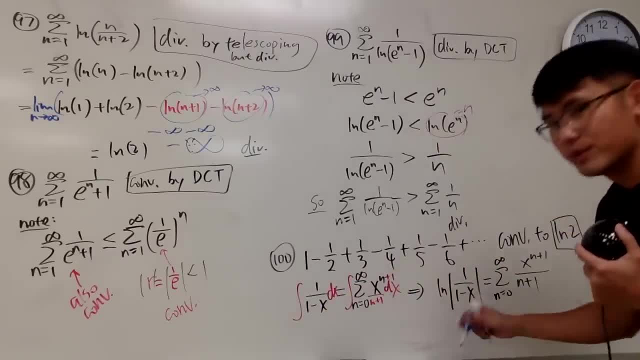 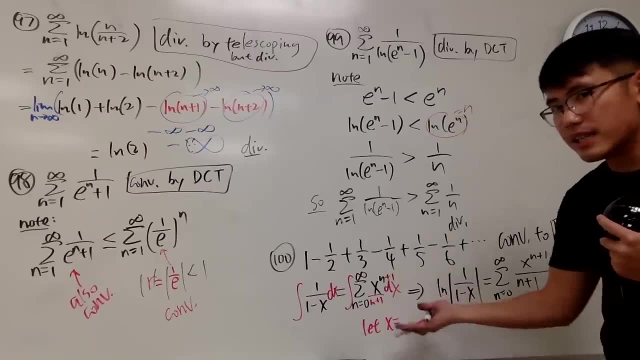 No, I'm going to finish it. I'm doing blue. well, I'm still doing black and red. Let x equal. I know there's another version, but I want to do this because this is the best friend version, right. 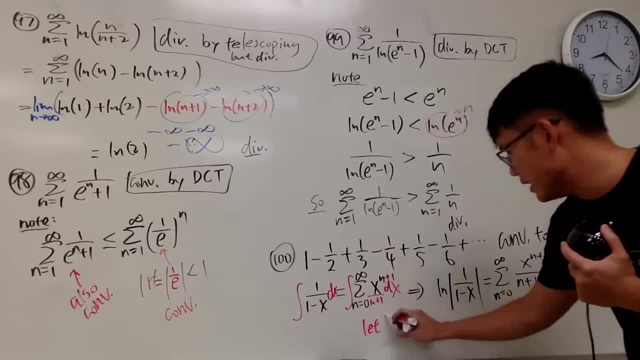 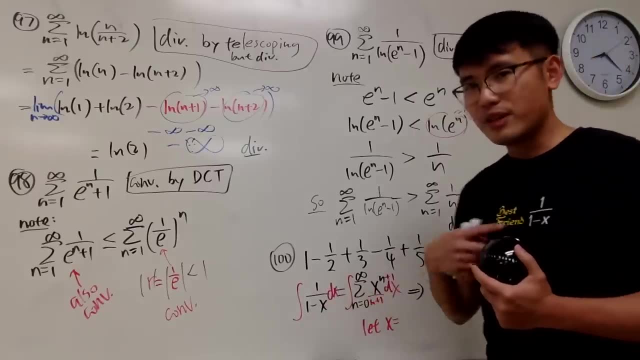 Well, I'm still doing black and red. Let x equal. I know there's another version, but I want to do this because this is the best friend version right. Integral of the best friend is the ln of the best friend right. 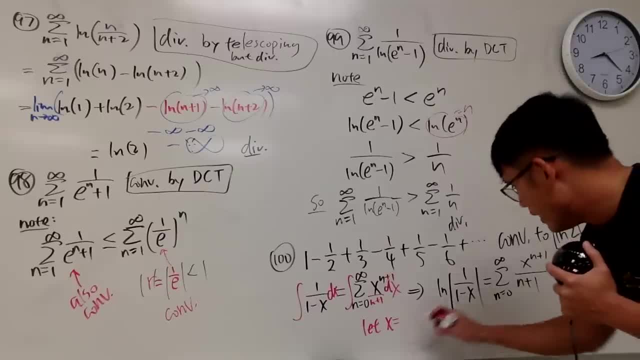 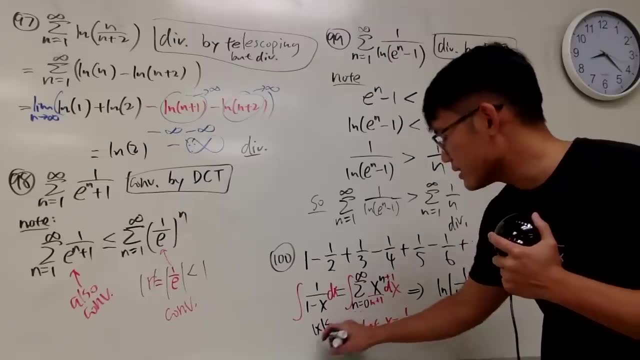 Integral of the best friend is the ln of the best friend. right. I will let x equal to 1 half And remember this is still a jet as long as x is the absolute value of x is less than 1, so this is still a jet. 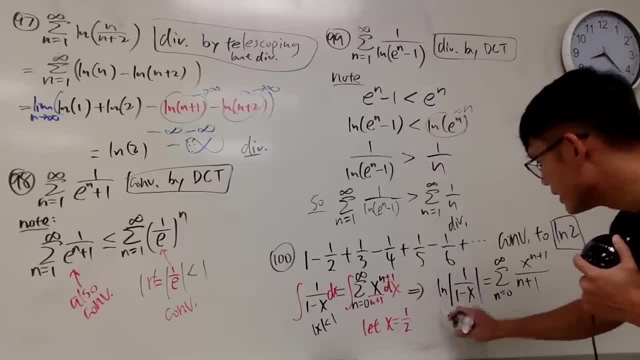 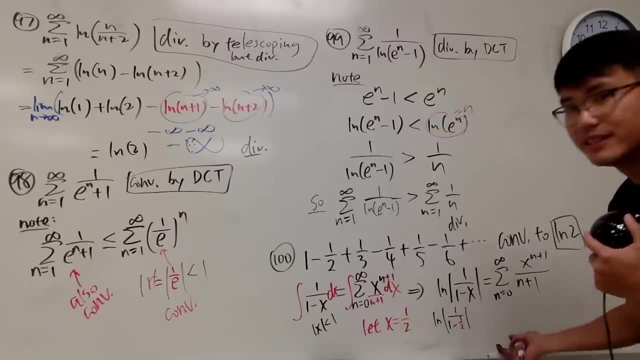 Put the 1 half in here, We end up with ln absolute value of 1 over 1 minus 1 half, like this right, And we just get this being equal to No, I don't want to use 1 half. 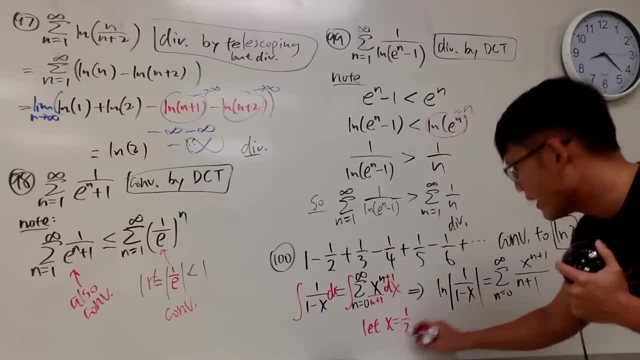 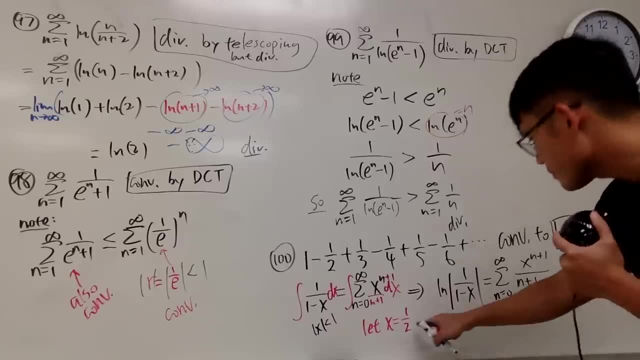 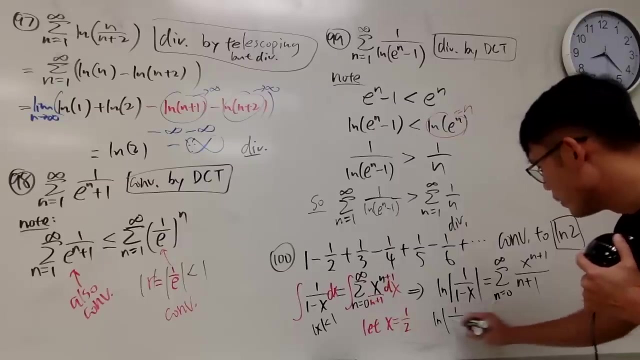 I will let x equal to 1 half And remember this is still a jet as long as x is Absolute value. of x is less than 1, so this is still a jet. Put the 1 half in here We end up with ln absolute value of 1 over 1 minus 1 half, like this right. 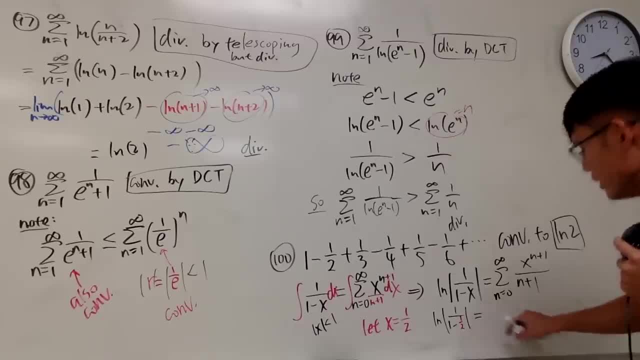 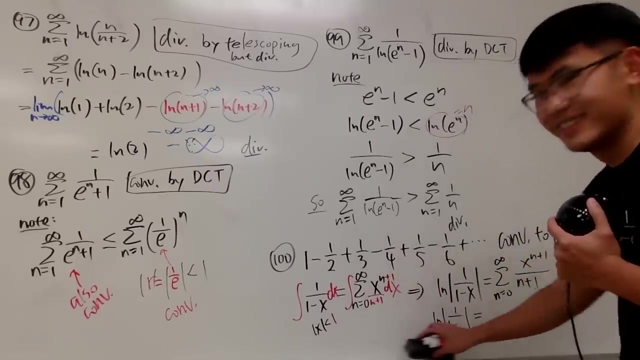 And we just get this being equal to No, I don't want to use 1 half. My bad, I don't want to use 1 half, I want to use negative 1.. All right, so here is the deal. 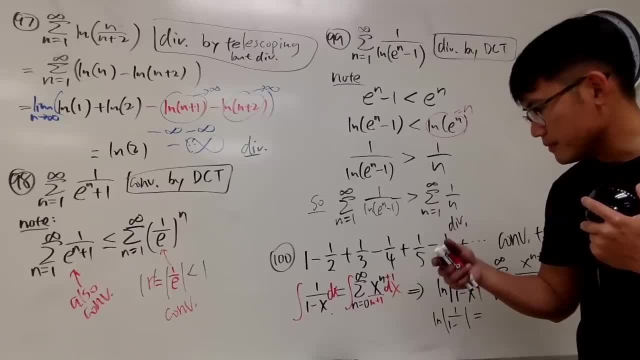 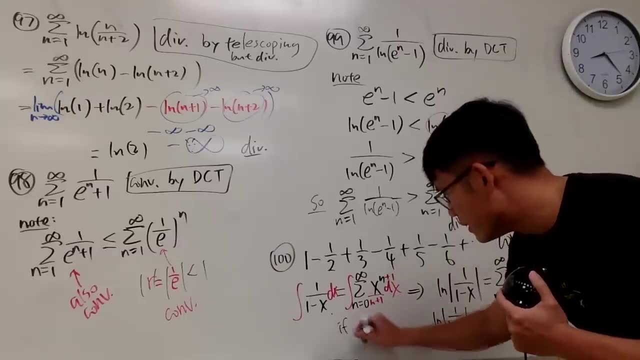 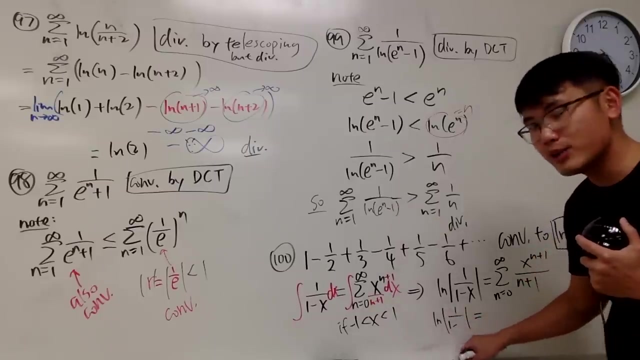 We talked about this earlier for the interval convergence for power series. right, This is actually true if. Let me just tell you, If x is in between of negative 1 and 1, but you have to pay attention to the endpoints. 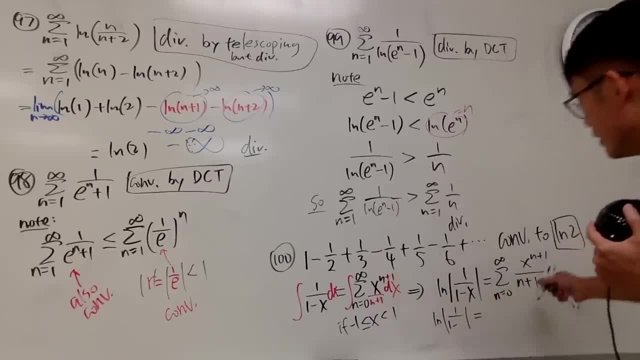 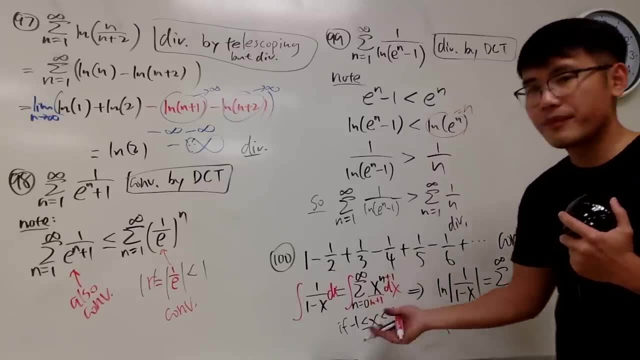 If you plug in negative 1 for x, you get an alternating series. So that's actually true, That's actually legit. So this right here is actually work for that Best friend. it's only going from negative 1 to 1 without the endpoints. 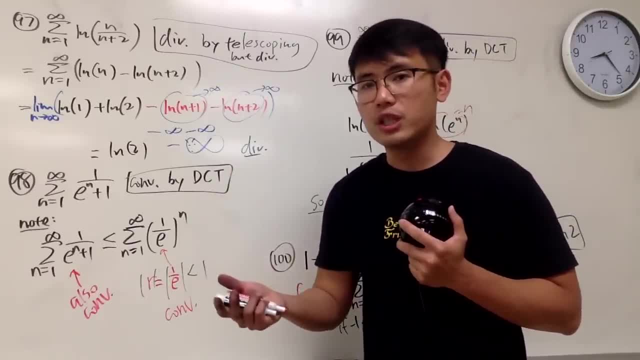 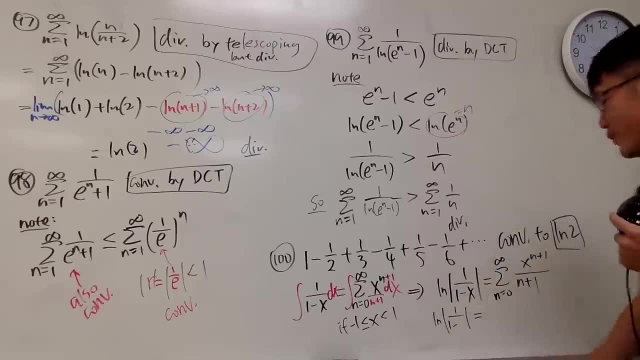 But when you differentiate it or when you integrate a power series, in general you have to double check the convergence at the endpoints. So we do happen to get to use negative 1 for this situation. So I will plug in negative 1 right here. 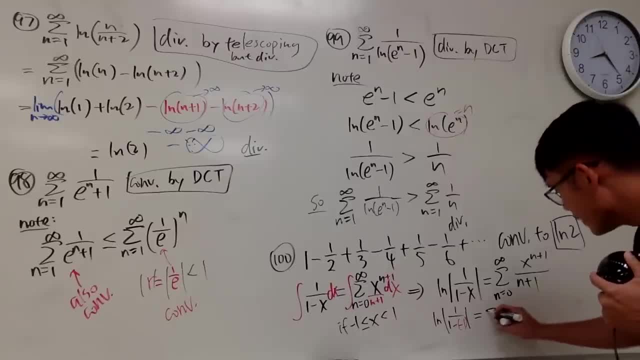 All right. And then, on the other hand, here we get the sum, as n goes from 0 to infinity, And then we get negative 1.. 12n plus 1 over n plus 1, like that. Now check this out. 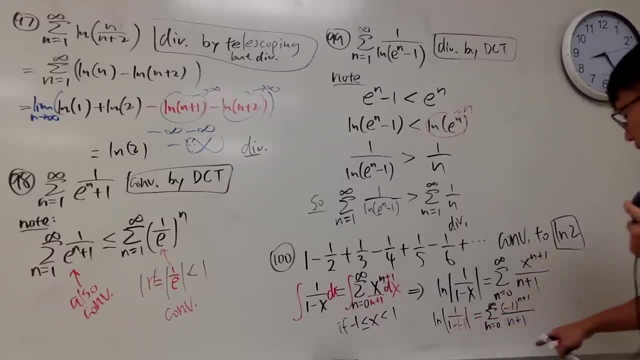 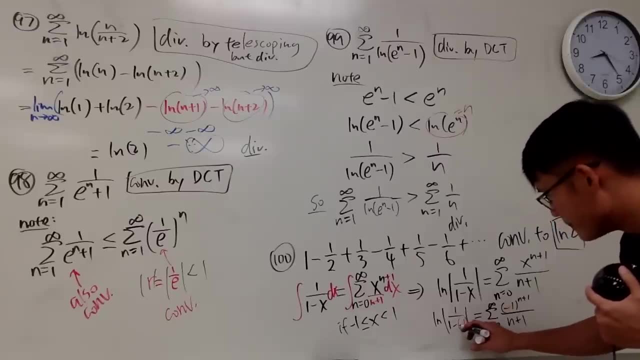 This is 2, right. And Why did I just? Why did I do this question right here? Let's see This right: here is 1 half. Well, by the log property we can write this as negative ln. 2, right. 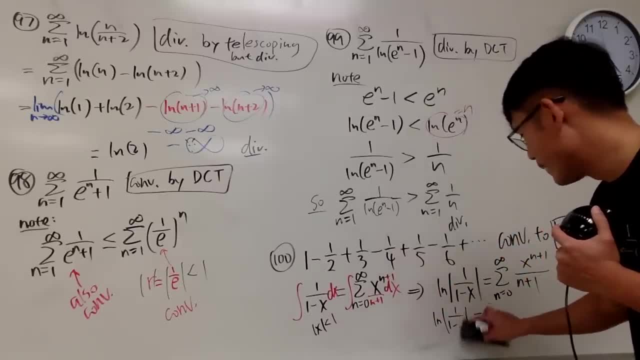 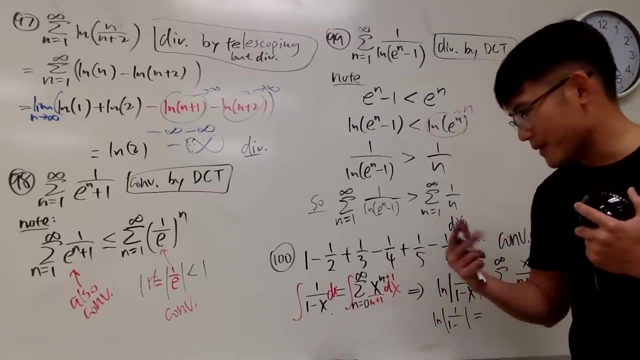 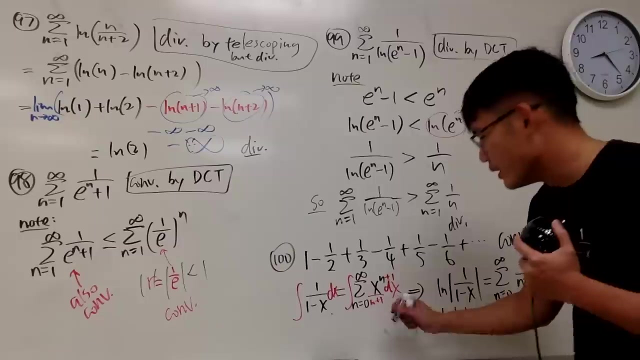 My bad, I don't want to use 1 half, I want to use negative 1.. Alright, so here is the deal. We talked about this earlier for the interval convergence for power series, right? This is actually true, if, let me just tell you. 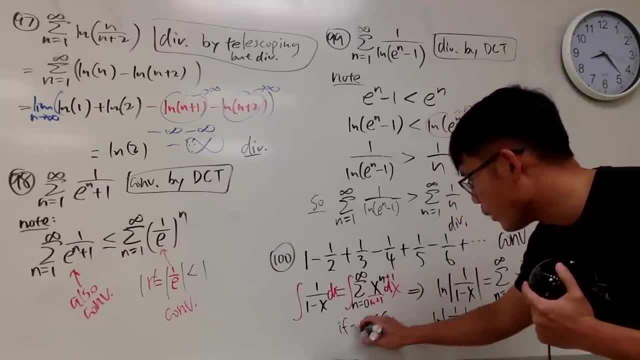 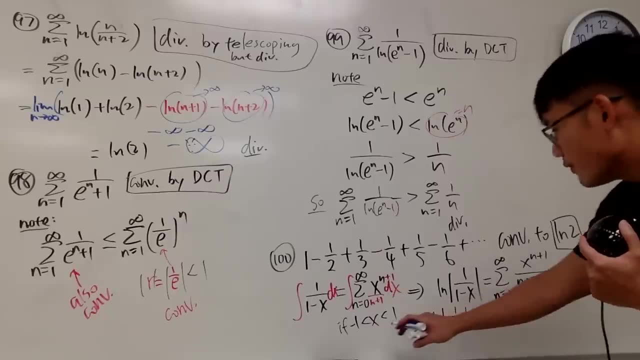 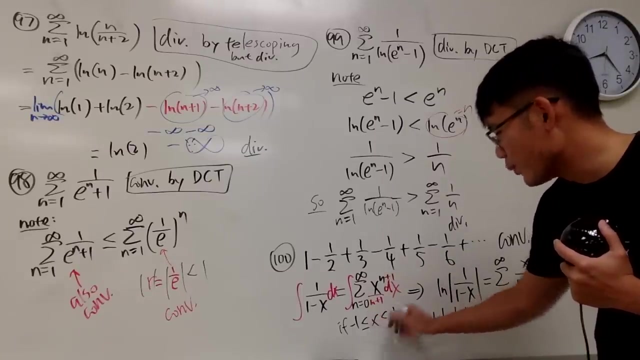 if x is in between of negative 1 and 1, but you have to pay attention to the endpoints. If you plug in negative 1 for x, you get an alternating series. So that's actually true, That's actually legit. So this right here is actually work for that. 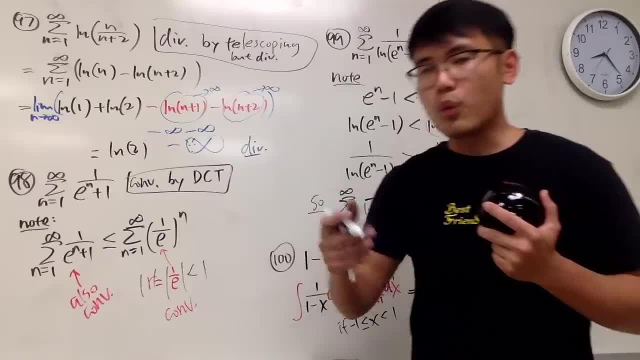 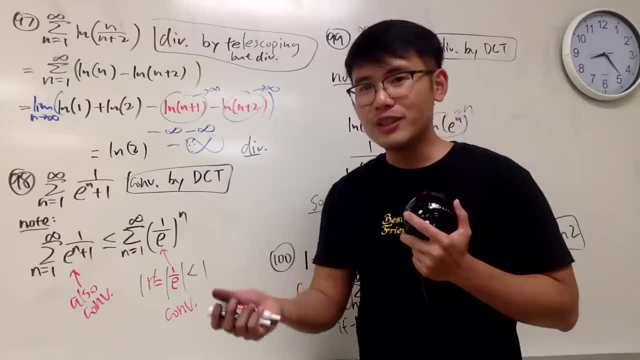 Best friend. it's only going from negative 1 to 1 without the endpoints. But when you differentiate it or when you integrate a power series, in general, you have to double check the convergence at the endpoints. So we do happen to get to use negative 1 for this situation. 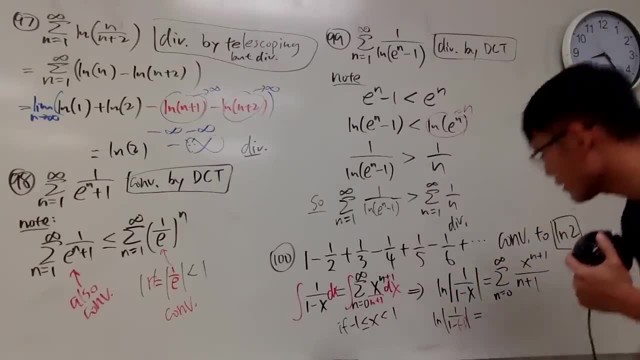 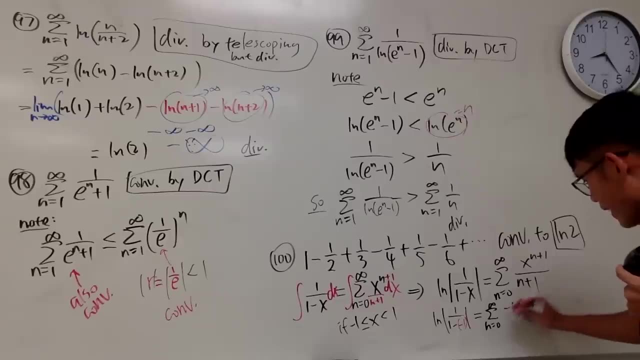 So I will plug in negative 1 right here, Alright. And then, on the other hand, here we get the sum as n goes from 0 to infinity, and then we get negative 1, n plus 1 over n plus 1,. 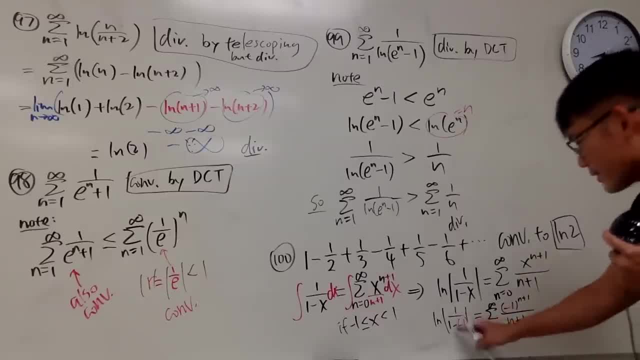 like that. Now check this out. This is 2, right, And why did I just? why did I do this question right here? Let's see This right: here is 1 half Well, by the log property. 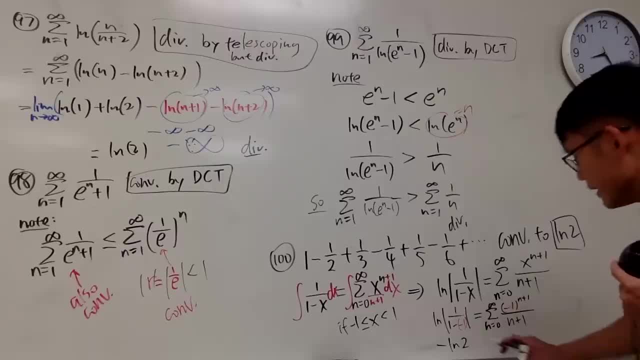 we can write this as negative ln 2.. Right This, right here. if you expand it, you get plug in 0, you get actually negative 1 to the first power, which is negative 1 over 1, because n goes from 0.. 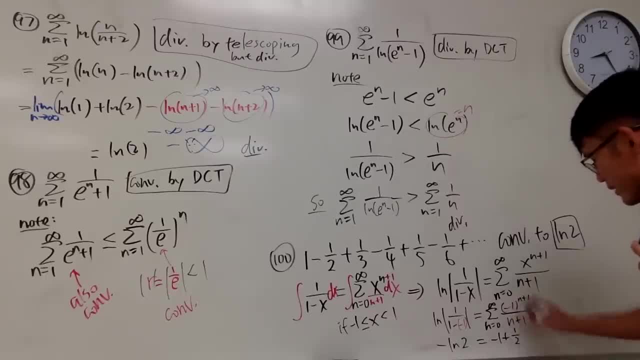 And then next you are going to add 1 over 2, and then next you are going to subtract 1 over 3, and next you are going to add 1 over 4, and so on, so on, so on. 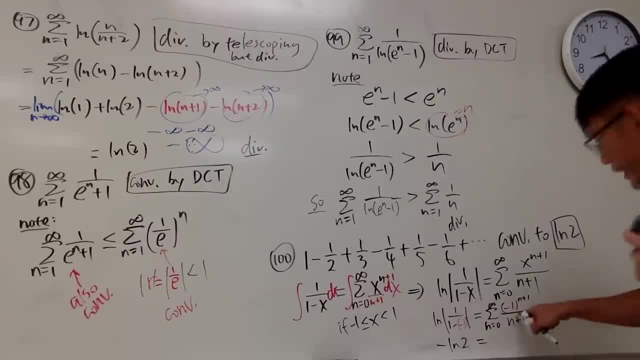 This right here. if you expand it, you get plug in 0, you get actually negative 1 to the first power, which is negative 1 over 1 because n goes from 0. And then next you are going to add 1 over 2.. 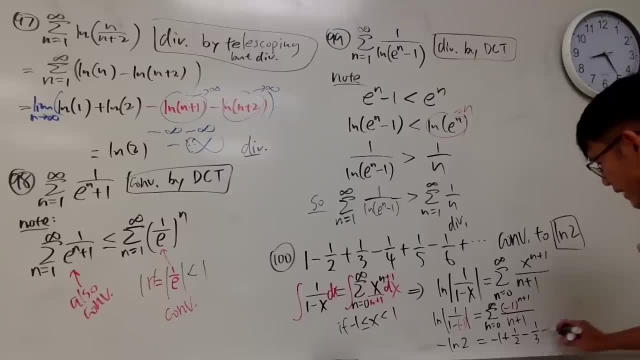 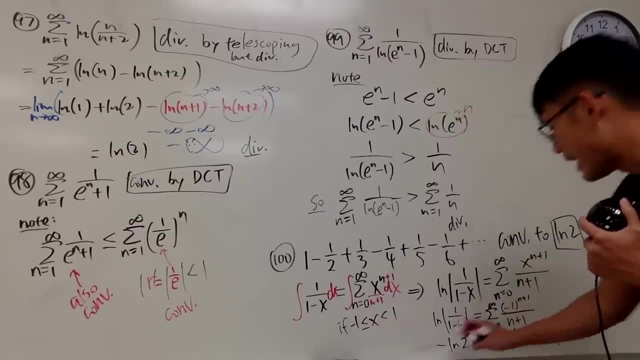 And then next you are going to subtract 1 over 3. And next you are going to add 1 over 4. And so on, so on, so on. But, as you can see, if you multiply both sides by negative 1.. 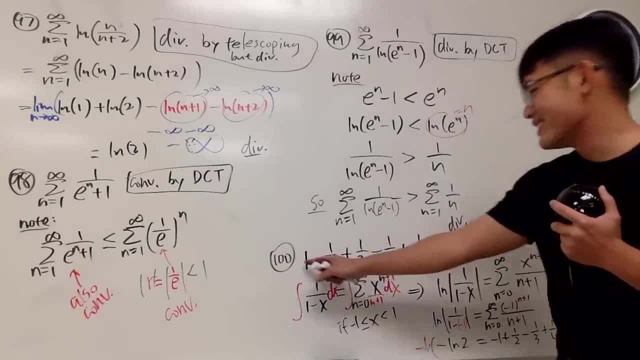 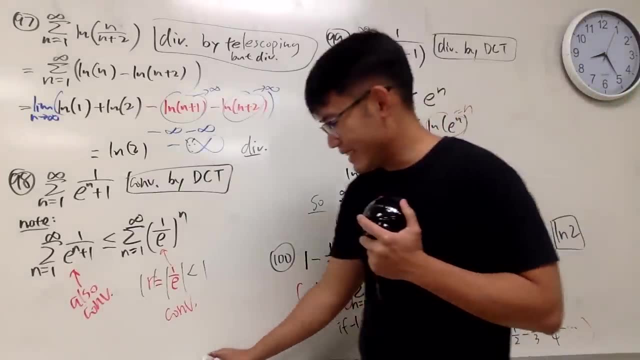 Yes, We did it This times. that is just ln 2. And, of course, the right-hand side is exactly that. So, So perfect, isn't it? That's it? huh, 100 questions. Yes, Of course, I have a bonus for you guys. 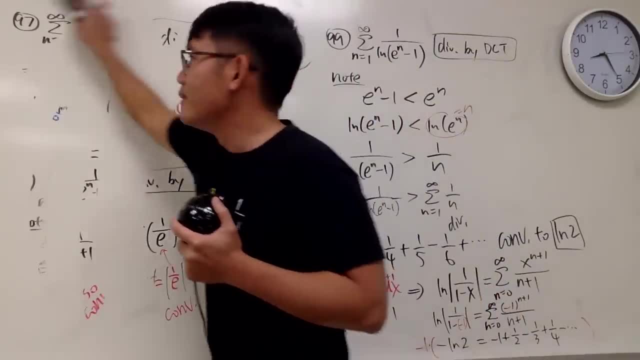 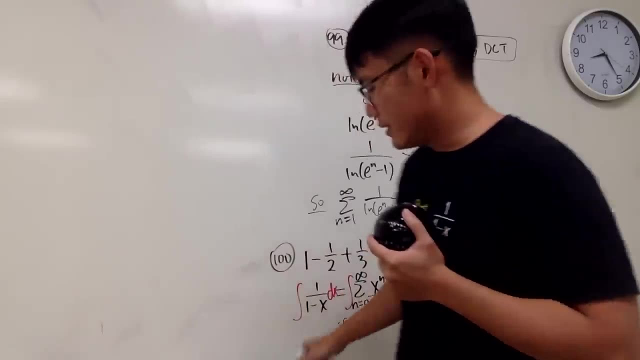 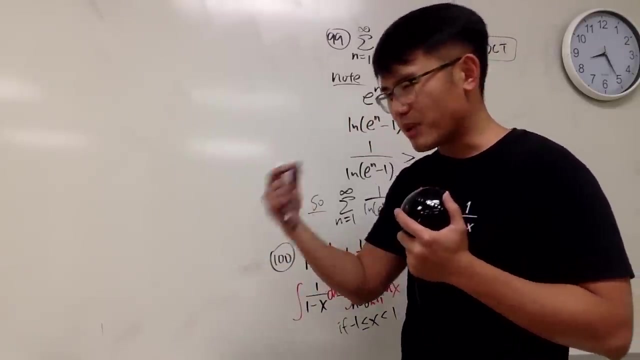 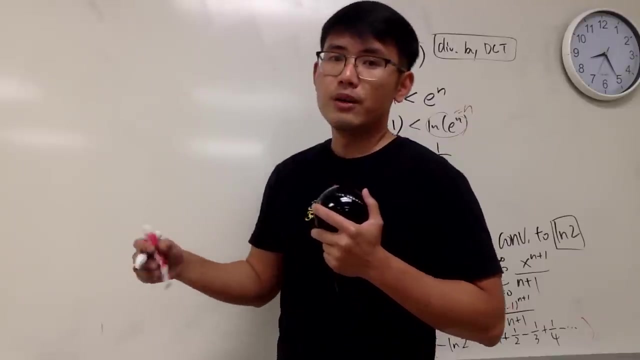 If you guys are watching it towards the end. So here is the DO. So far we have compared power function and exponential and tried to compare them with, tried to team them up and compare with factorial, But it didn't work. So 101, this is what we are going to do. 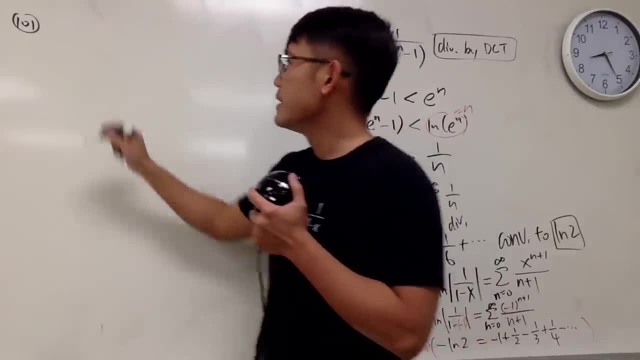 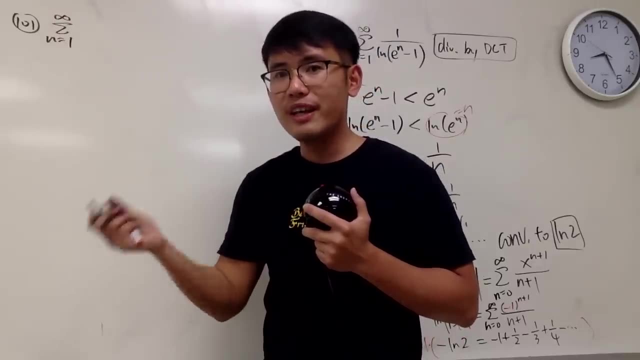 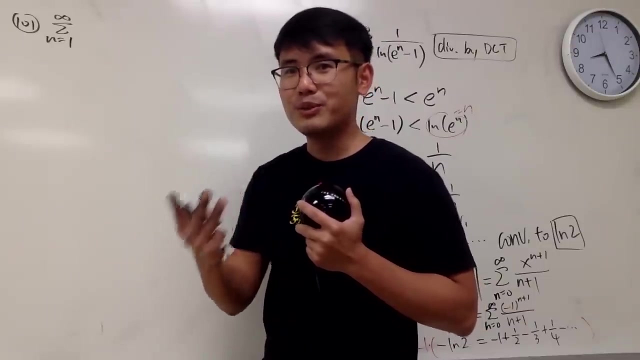 We are going to compare What if we have the sum as n goes from 1 to infinity? I want to team them up with a power function and also a factorial, And n to the n Right. So pretty much the first, The biggest 3x. 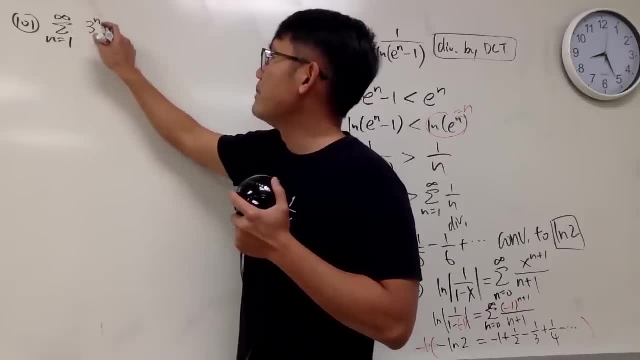 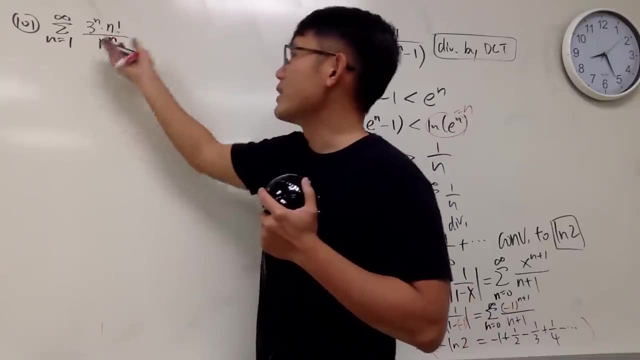 Right. So anyway, let me tell you guys, 3 to the n times n factorial, And we'll compare this with n to the n, We'll divide it by. We'll try to compute that, Okay. So here we'll do the ratio test. 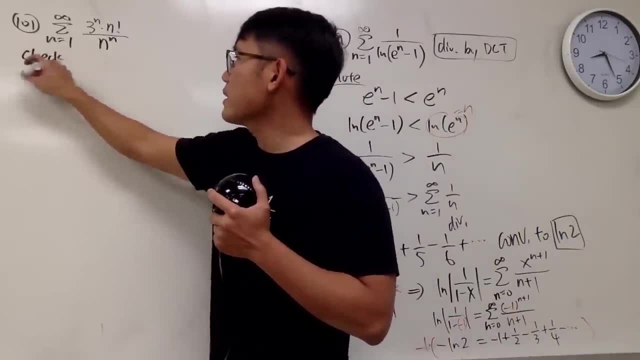 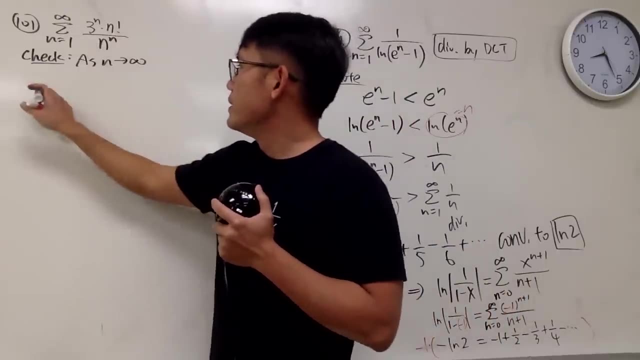 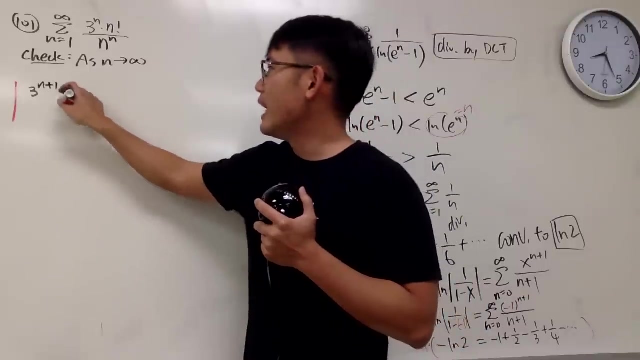 So let's go ahead and check s n goes to infinity. Okay, here we go. Here we have to take the absolute value, So it doesn't really matter Because everybody is positive. So do this, And then you have n plus 1 factorial. 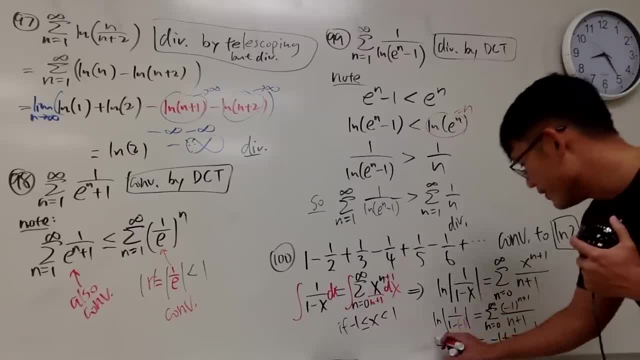 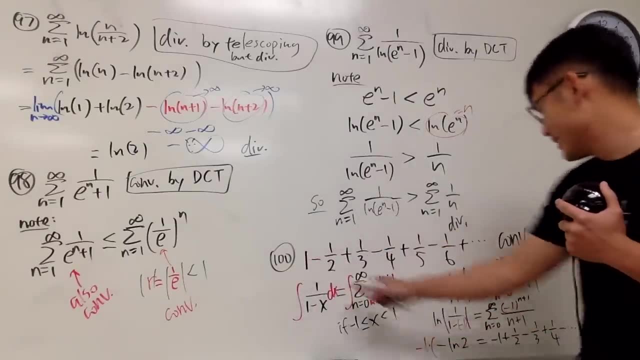 But, as you can see, if you multiply both sides by negative 1,- yes, we did it This times- that is just ln 2. And, of course, the right hand side is exactly that. So, so perfect, isn't it? 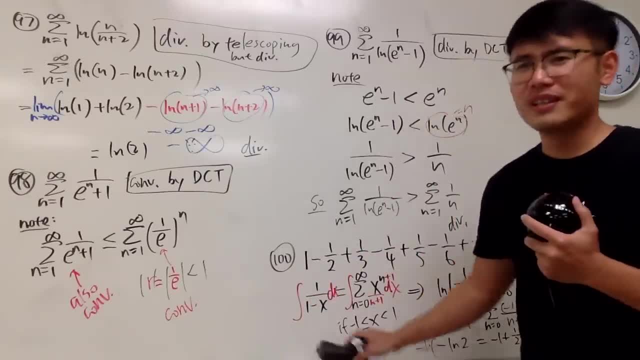 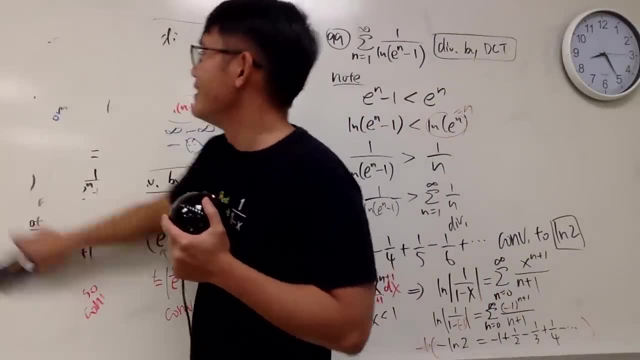 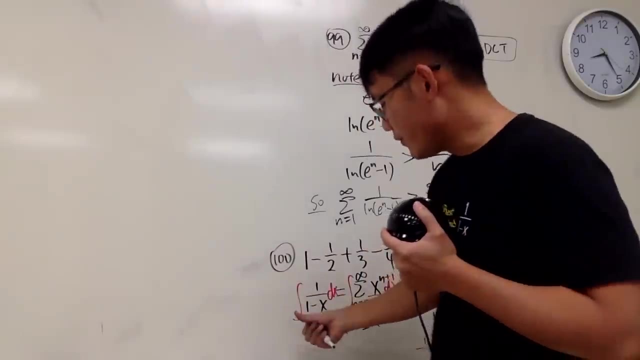 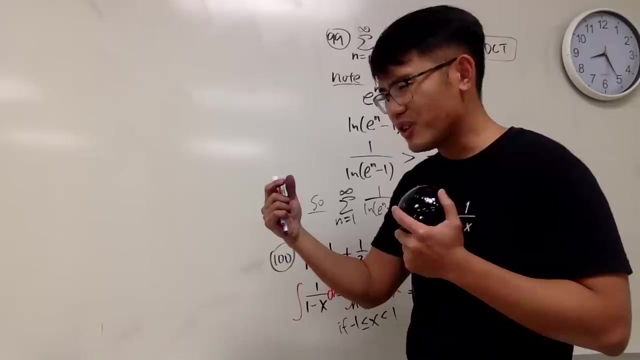 That's it. huh, 100 questions. Yes, Of course I have a bonus for you guys if you guys are watching it toward the end. So here is the deal. So far we have compared power function and exponential. 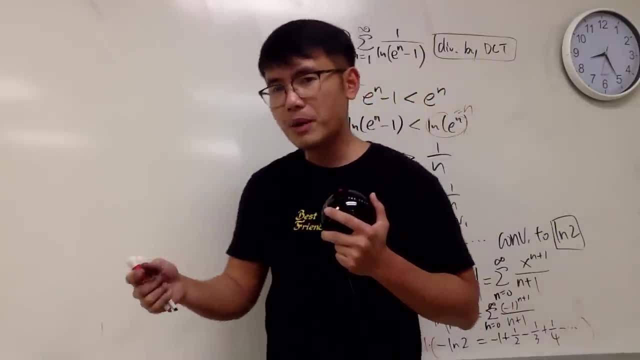 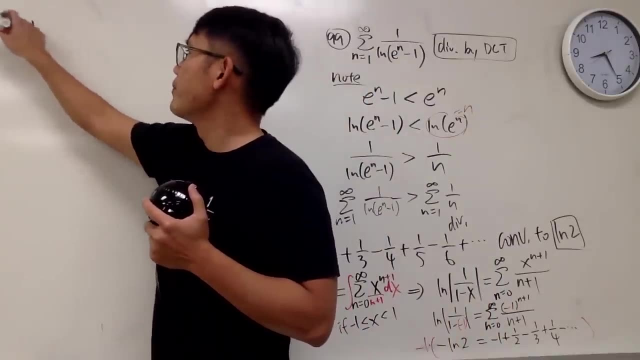 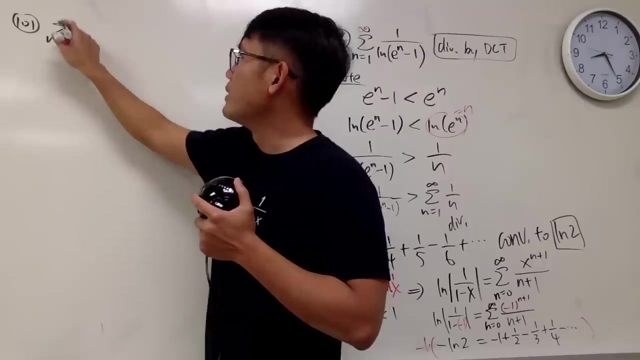 and tried to compare that with, tried to team them up and compare with factorial, but didn't work. So 101, this is what we are going to do. We are going to compare what if we have the sum as n goes from 1 to infinity. 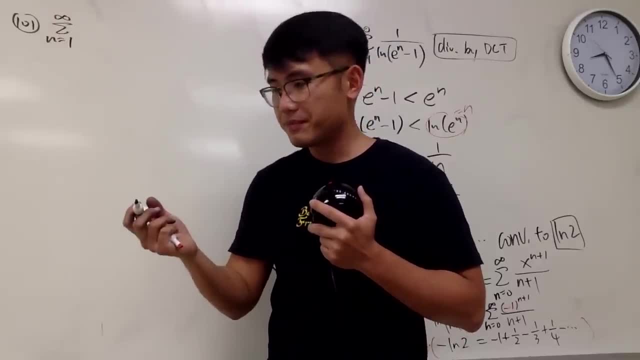 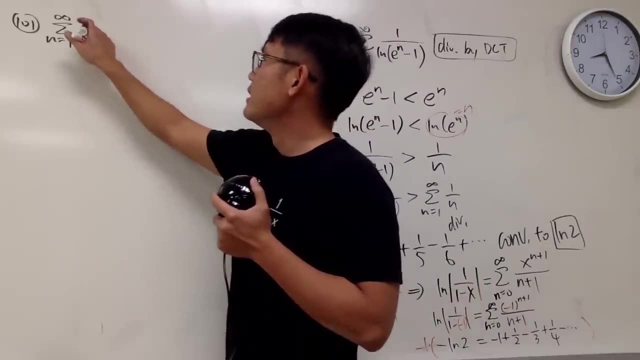 I want to team up with the power function and also factorial and n to the n. So pretty much the first, the biggest 3x Right? So anyway, let me take this 3 to the n times n factorial. 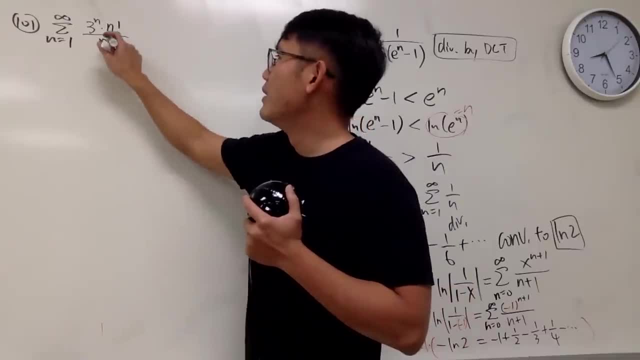 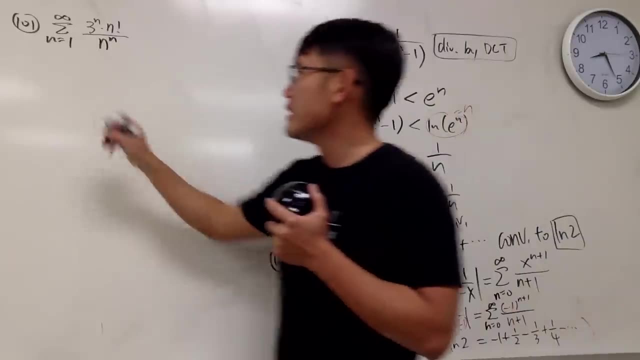 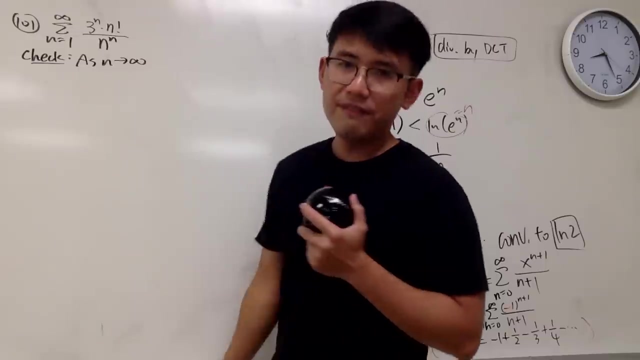 and we'll compare this with n to the n. We'll divide it by. you know, we'll try to compute that, Okay. So here we'll do the ratio test. So let's go ahead and check. S n goes to infinity. 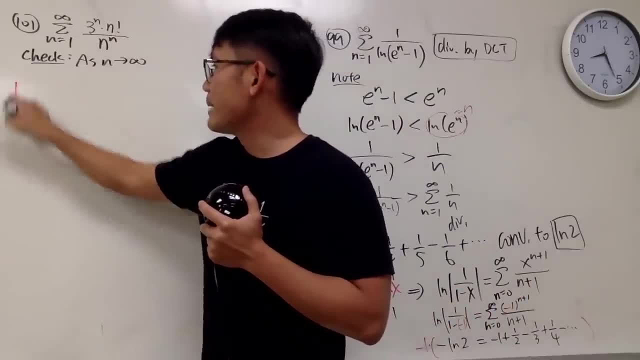 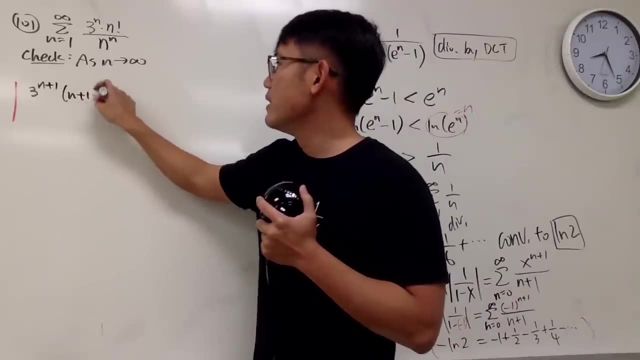 Okay, here we go. Here we have to take the absolute value, so it doesn't really matter because everybody is positive. So do this, and then you have n plus 1 factorial and then over n plus 1 to the n plus 1 power. 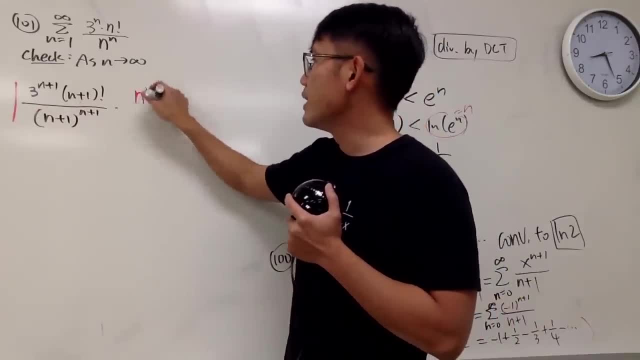 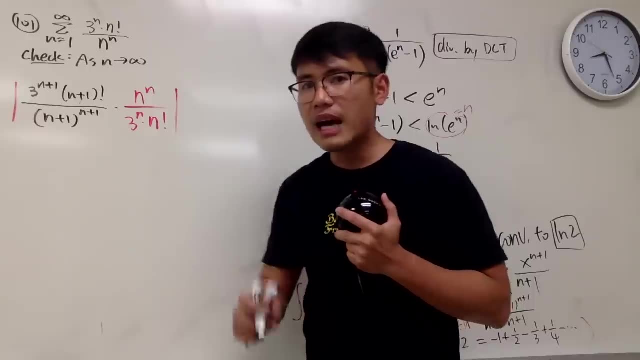 times do the reciprocal, we get n to the n, over 3 to the n n. factorial Absolute value of that. Now here is the deal: Clean up the factorials of the business. This is 3 to the n. 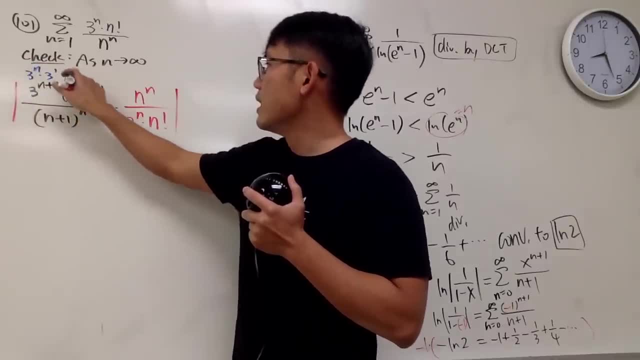 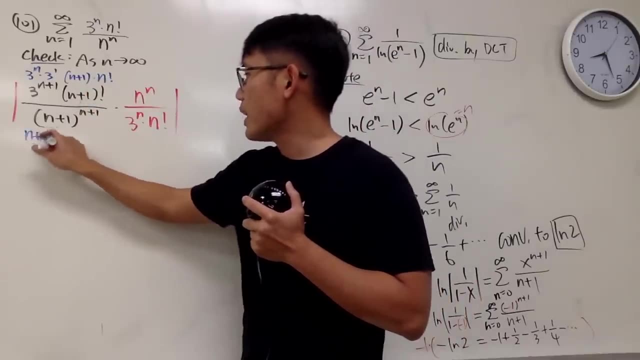 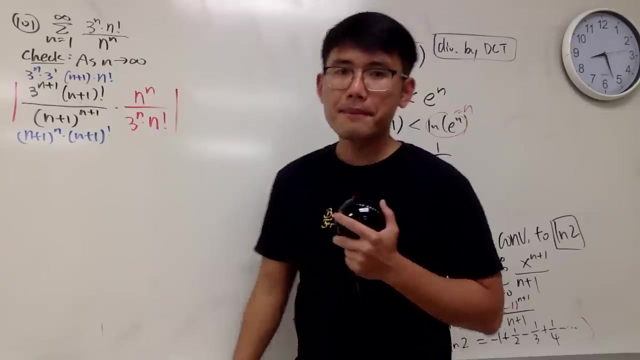 times 3 to the first. this, right here, is n plus 1, times n factorial, and this, right here is n plus 1, to the n times n plus 1, to the 1, like this. Okay, So, as we can see right here, 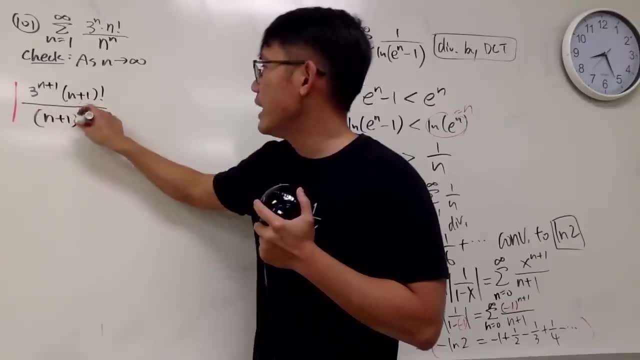 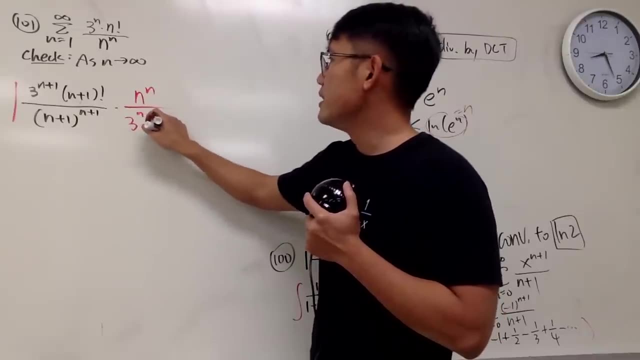 And then over n plus 1 to the n plus 1.. N plus 1 to the n plus 1 power times Do the reciprocal. We get n to the n over 3 to the n n factorial Absolute value of that. 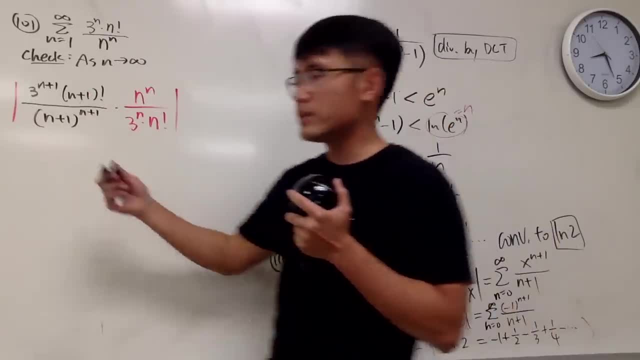 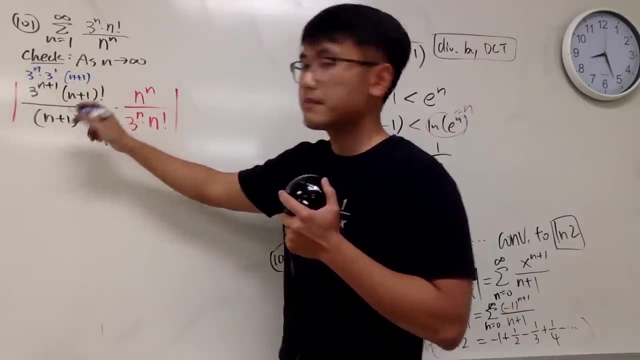 Now here is the deal: Clean up the factorials of the business. This is 3 to the n times 3 to the first. This right here is n plus 1 times n factorial. And this right here is n plus 1 to the n. 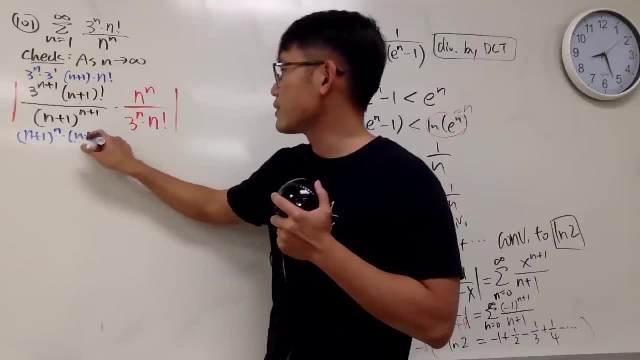 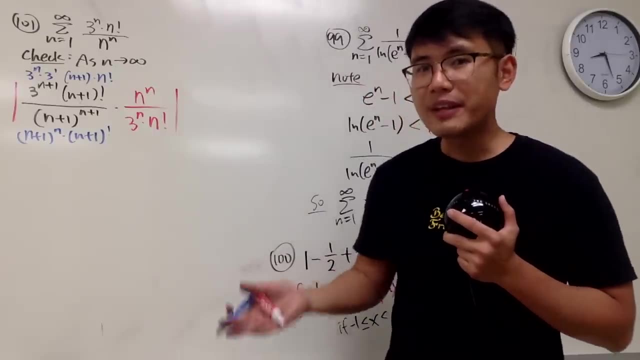 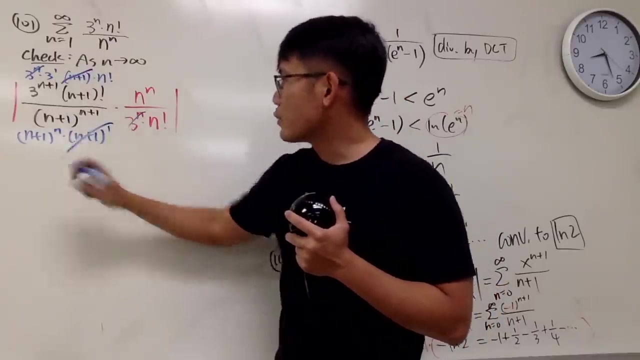 And this right here is n plus 1 to the n, times n plus 1 to the 1.. Like this, Okay. So, as we can see right here, 3 to the n, 3 to the n- cancel, And we have n plus 1, n plus 1, cancel. 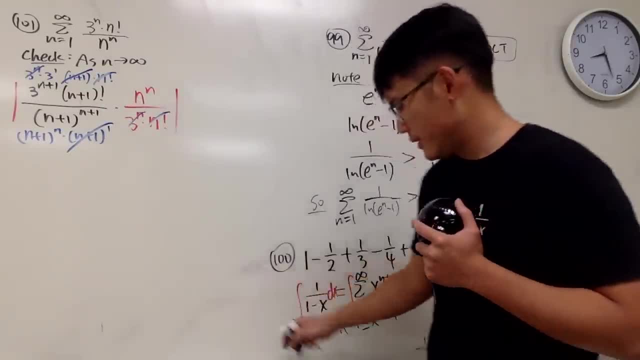 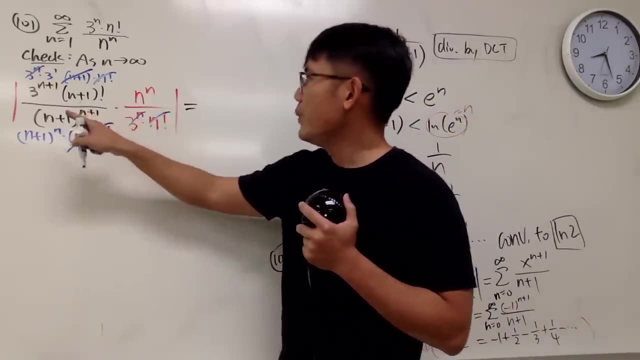 n factorial, n factorial cancel. And what do we end up with? In this case, it's a really nice competition. You will see, This, right here is equal to Okay, we have a street Right here. okay, We have a street okay. 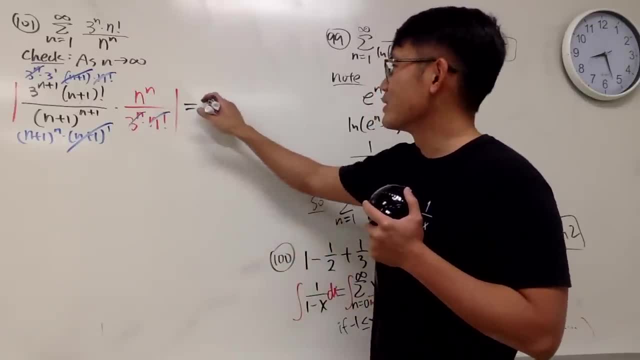 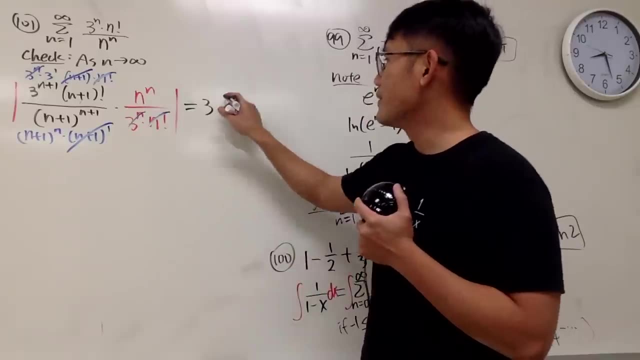 So we have a street and absolute value doesn't matter. You know that. So we have a street And again we have parentheses. Okay, let me just do this again to be formal. We have n to the n over n, plus 1 to the n. 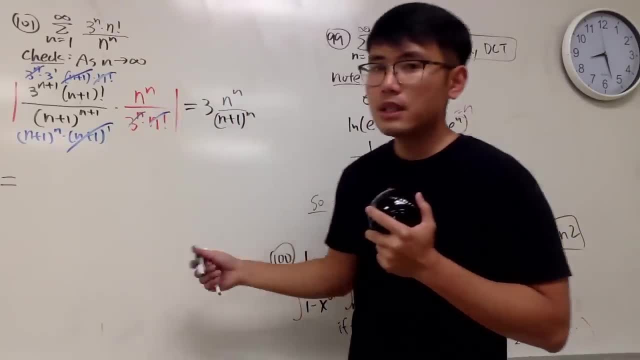 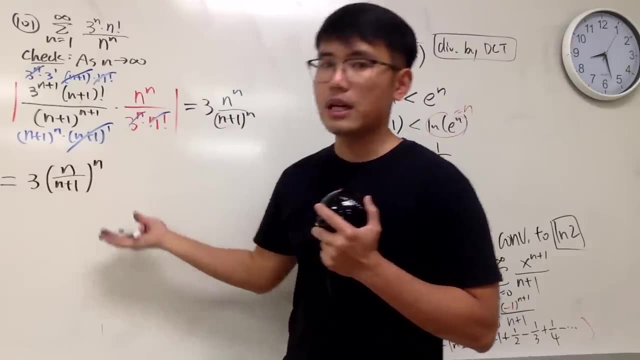 Right Now we're just going to do more algebra right here. Well, I'm just going to combine So we get 3 times n over n plus 1. And put the exponent on the outside. But hopefully by now you guys should know. 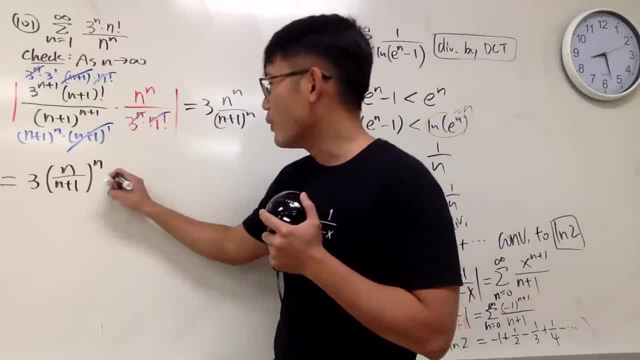 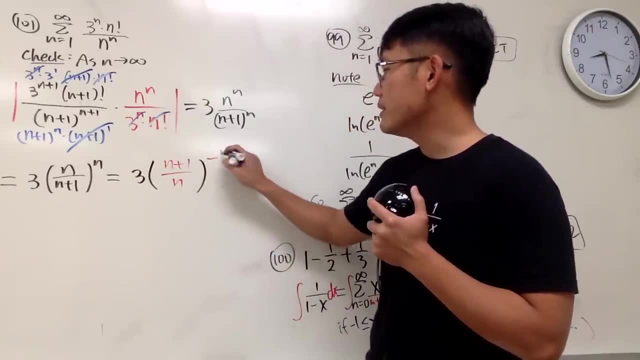 We will have to use the fact To do so. we will look at this as 3 times n plus 1 over n And make that into a negative exponent like this: And then, as you can see, we're still doing algebra. 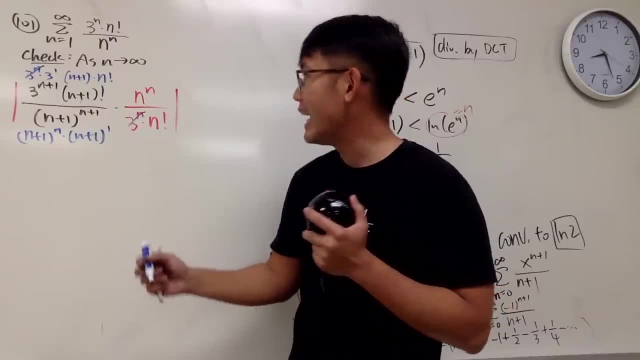 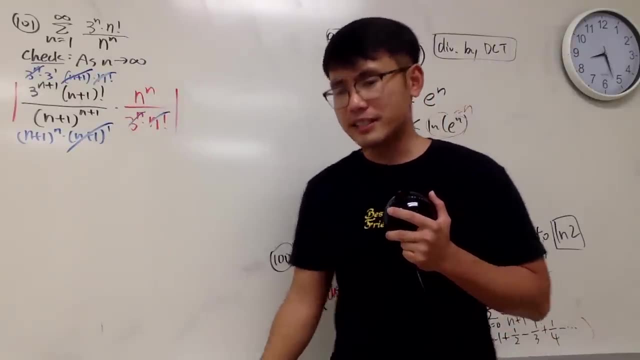 3 to the n, 3 to the n cancel, and we have n plus 1, n plus 1, cancel, n factorial, n factorial cancel. and what do we end up with In this case? it's a really nice competition. 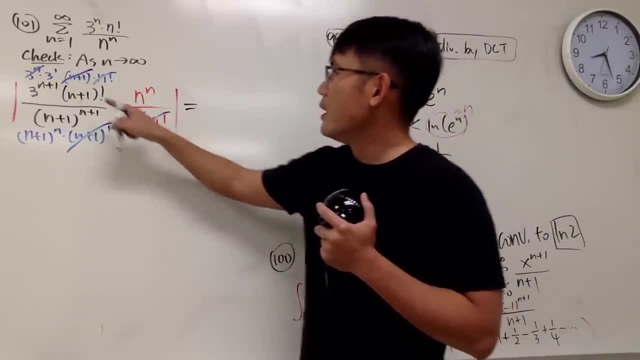 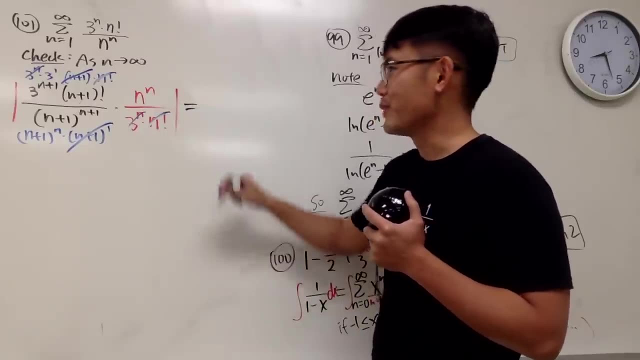 you will see This: right here is equal to: okay, we have a street right here. okay, we have a street. okay, So we have a street and absolute value doesn't matter. you know that. So we have a street. 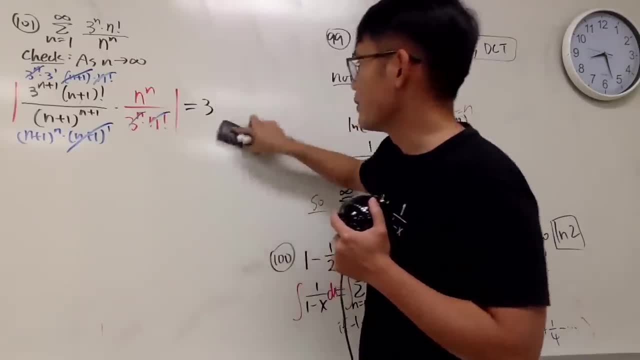 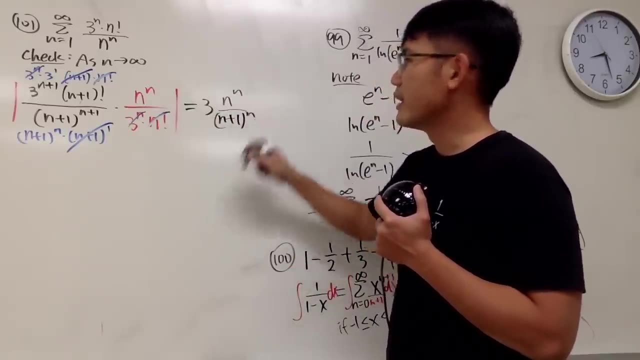 And again we have parentheses. okay, this is again to be formal. We have n to the n over n plus 1, to the n. right Now. we're just going to do more algebra right here. 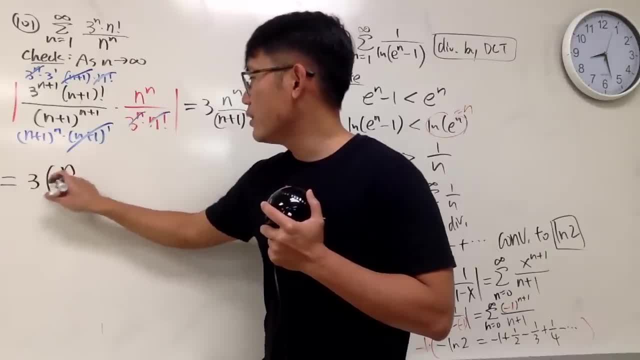 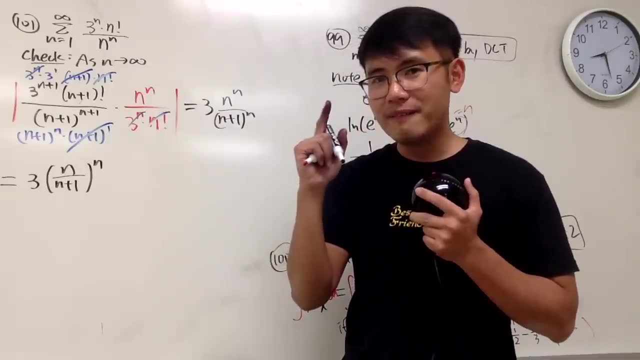 Well, I'm just going to combine so we get 3 times n over n plus 1, and put the exponent on the outside. but hopefully by now you guys should know we will have to use the fact. 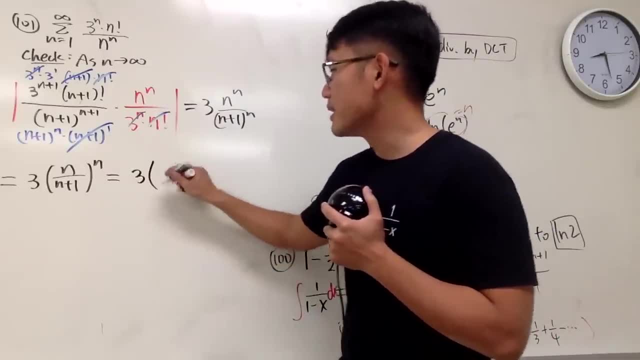 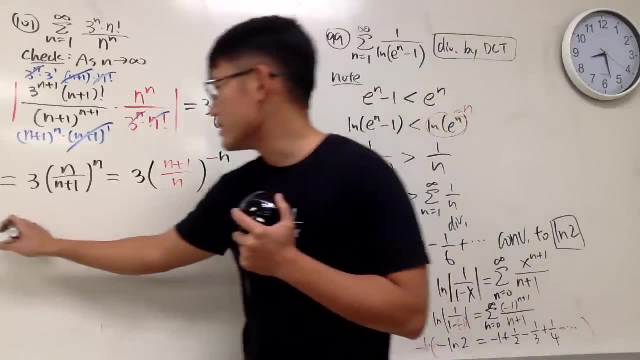 To do so, we will look at this as 3 times n plus 1, over n and make that into a negative exponent like this: And then, as you can see, we're still doing algebra. This is 3 times. 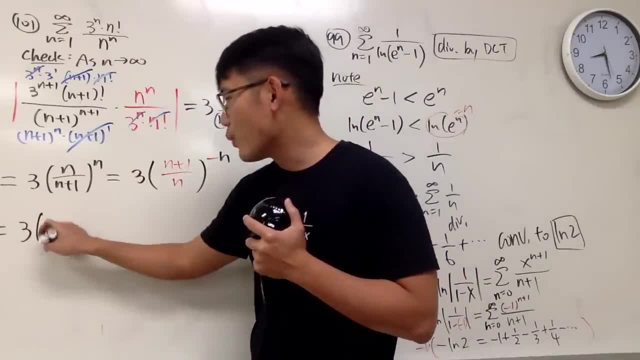 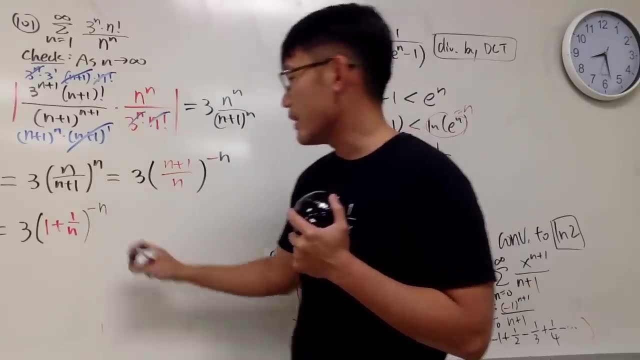 flip, I mean split, split. We get 1 plus 1 over n raised to the negative n power, like this: Okay, Take the limit, 3 is 3.. But this guy, well, a is. 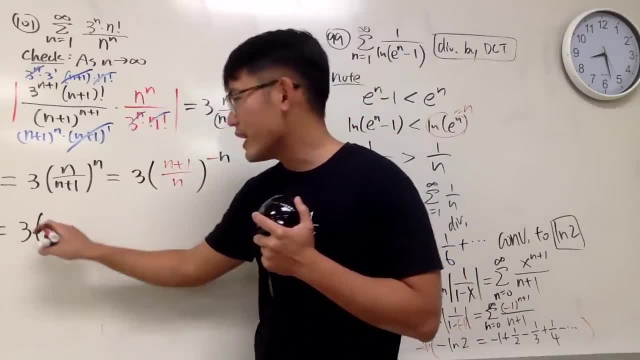 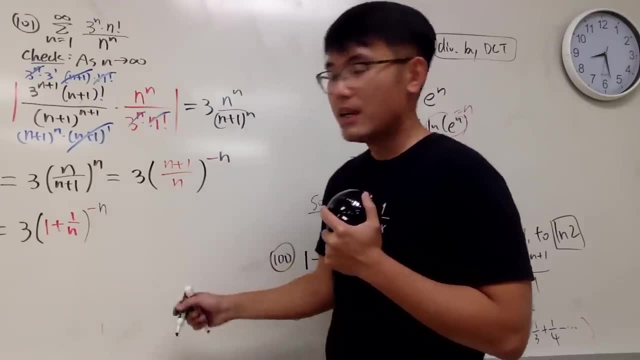 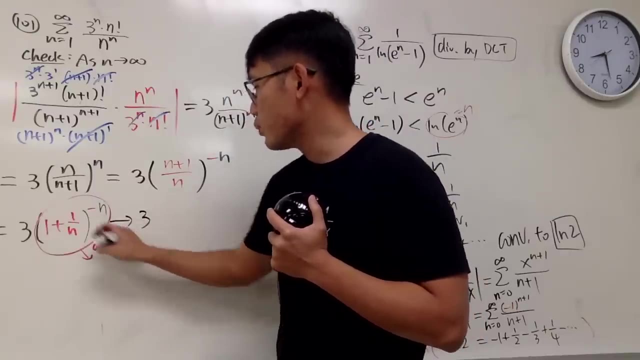 This is 3 times split. We get 1 plus 1 over n, raised to the negative n power like this: Okay, Take the limit, 3 is 3.. But this guy? Well, a is positive, 1.. b is negative, 1.. 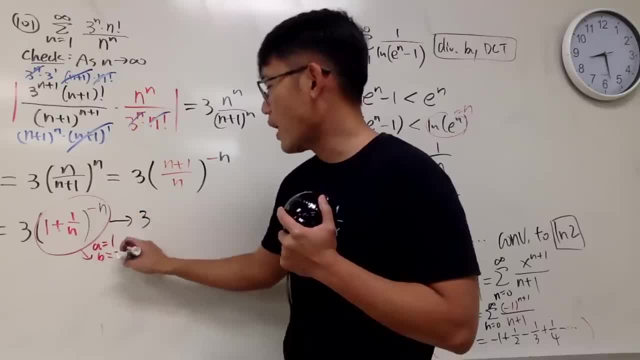 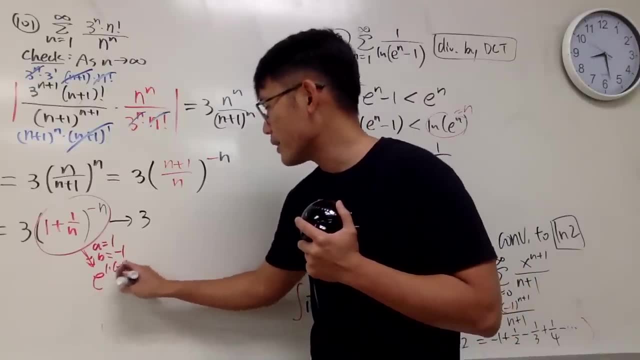 positive 1, b is negative 1.. So all in all this right here is e to the 1 times negative 1.. So in another word, this right here we have to multiply by 1 over e. 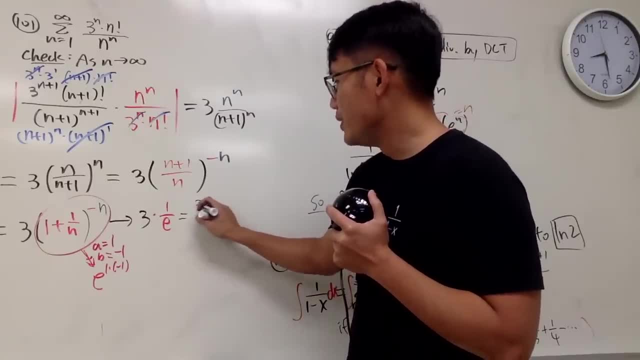 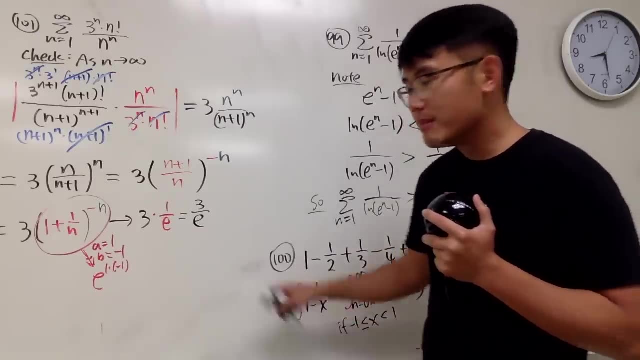 Ah, you see this right here is actually 3 over e. Oh my god, this is so fun Because you see this right here. e is about 2.7 something, 3 over e. 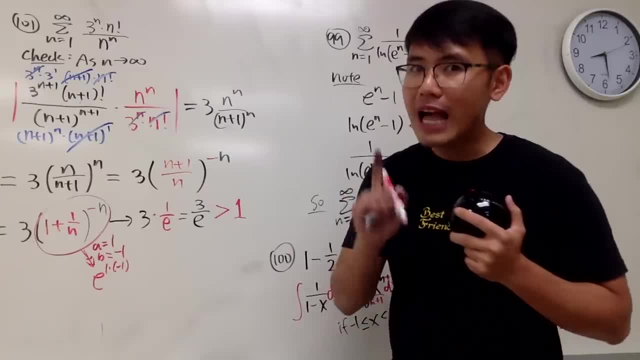 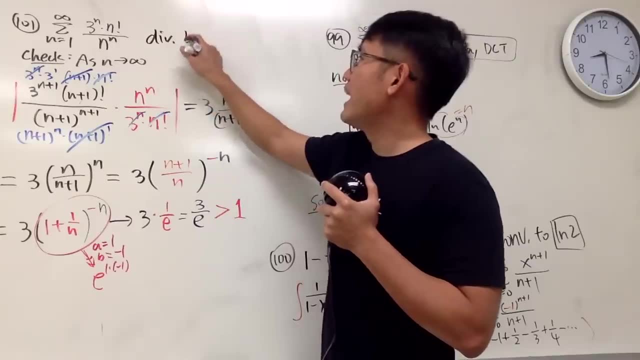 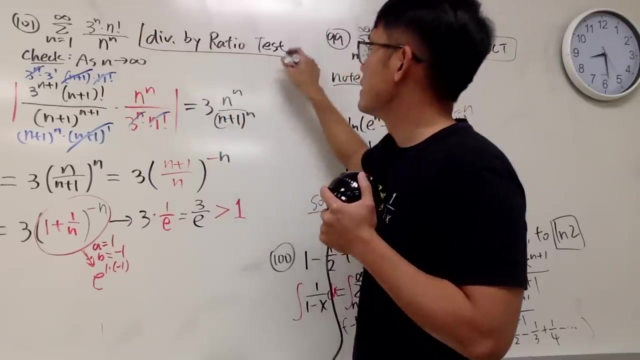 is actually bigger than 1.. So that means this guy right here diverges By ratio test. Okay, And you might wonder, is it always true if you pair up a power with? 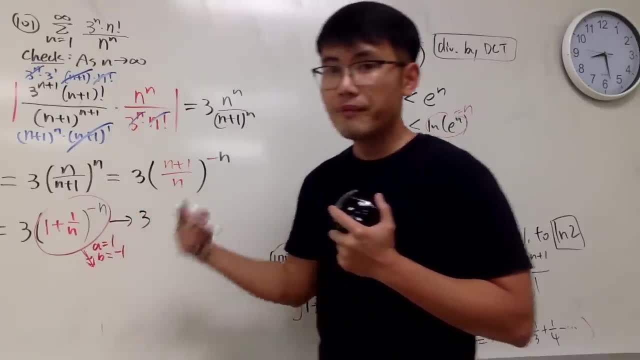 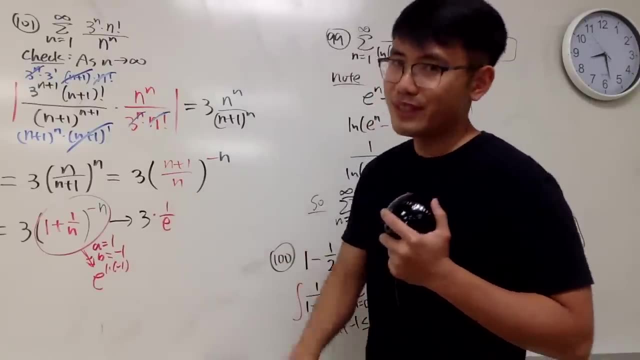 So, all in all, this right here gives us e to the 1 times negative 1.. So, in another word, this right here we have to multiply by 1 over e. Ah, you see, This right here is actually 3 over e. 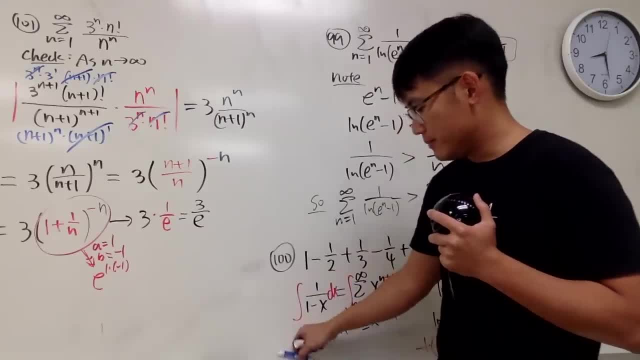 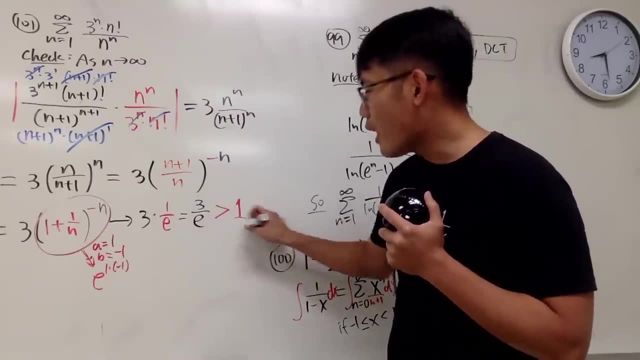 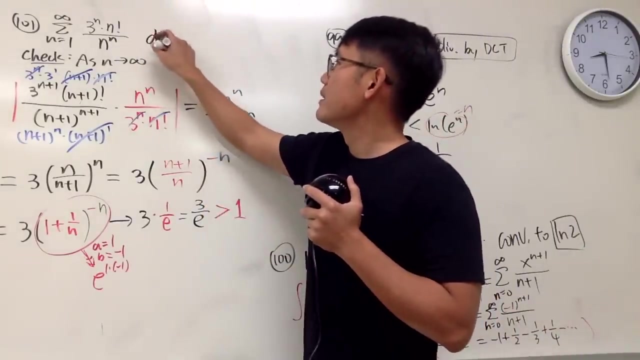 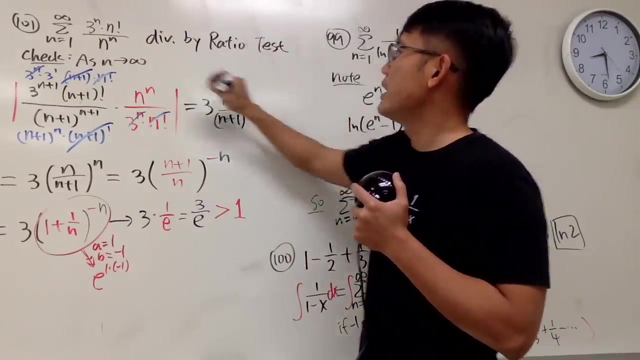 Oh my god, This is so fun Because you see This right here: e is about 2.7, something 3 over e is actually bigger than 1.. So that means this guy right here diverges by ratio test. 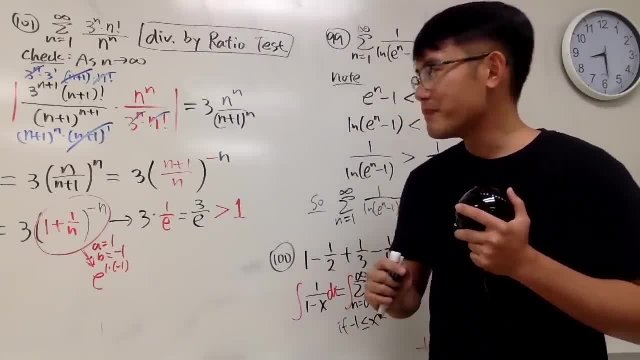 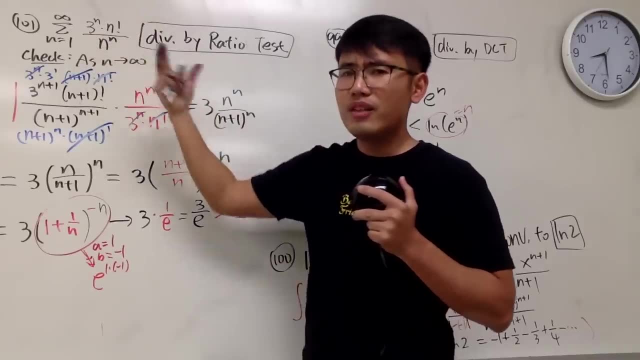 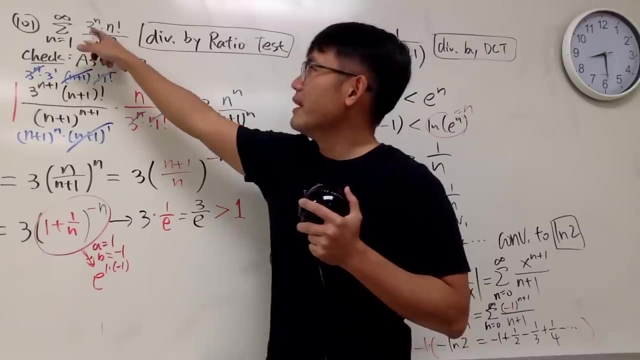 Okay, And you might wonder: Is it always true? If you pair up a power with factorial and divide it by n to the n, That will always going to be divergent, Maybe not? Why don't you just try 2 to the n and so on? 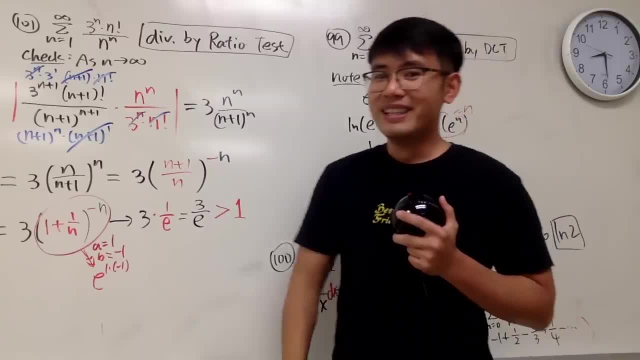 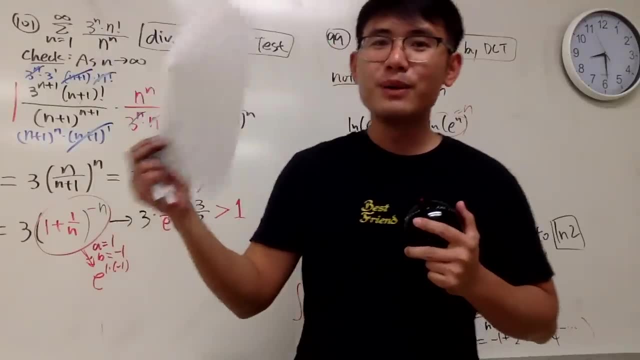 And leave a common number to let me know what the answer is. Anyway, Oh my god, Oh my god, I'm done. I'm done with all the questions, I'm done with all the questions. Oh my goodness. 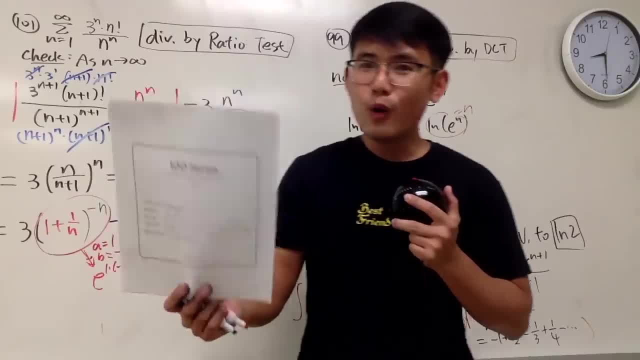 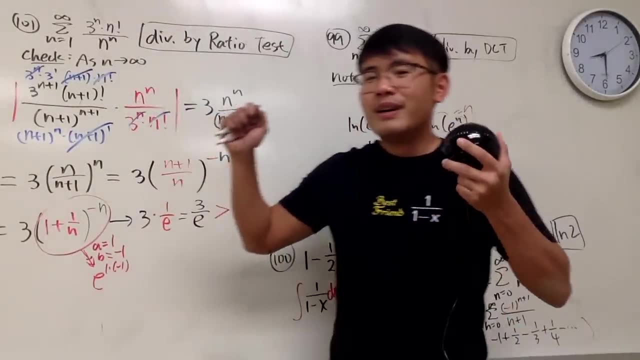 Oh my goodness. No food, No water, No stop. Okay, I just had to send a text message earlier, But you know That shouldn't be counted as a stop. Yes, My arms are so, So tired. All right, 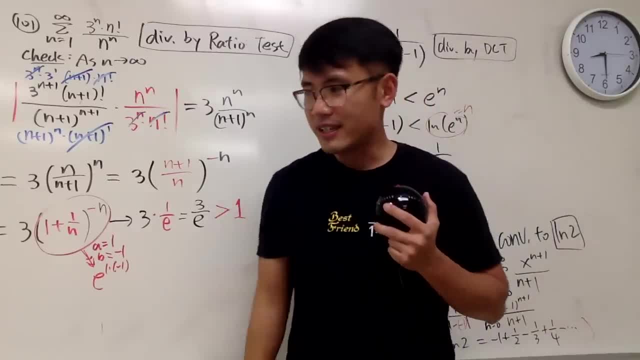 So hopefully you guys all find this video to be helpful. Seriously, Seriously. If you have any questions, just leave a comment down below. Let me know, And I hope you guys have a good day. Bye-bye, Bye-bye. 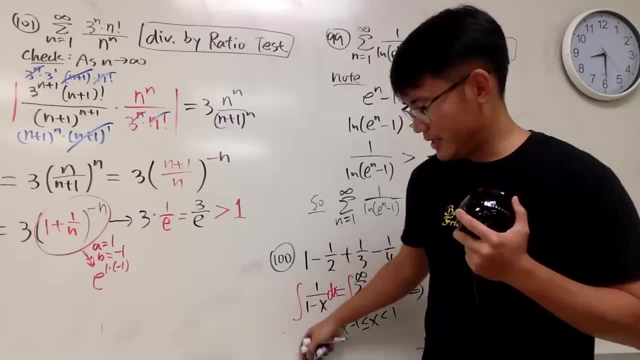 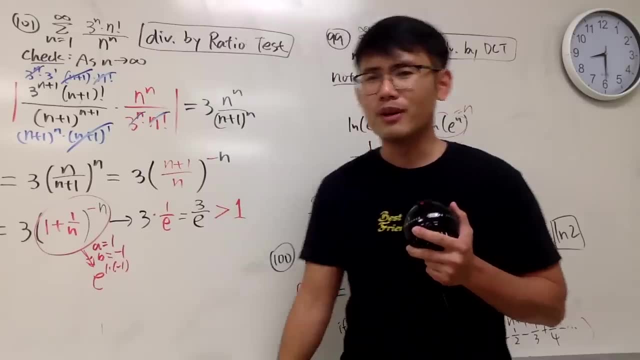 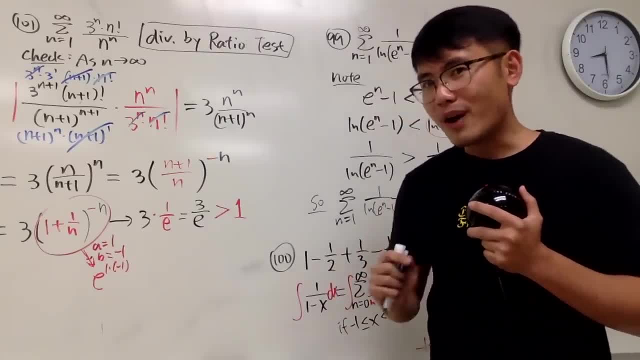 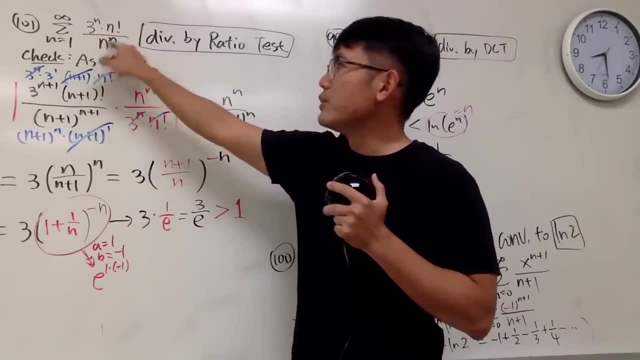 factorial and divided by n to the n, that will always going to be divergent, Maybe not? Why don't you just try 2 to the n, and so on? So this is a 2 to the n. 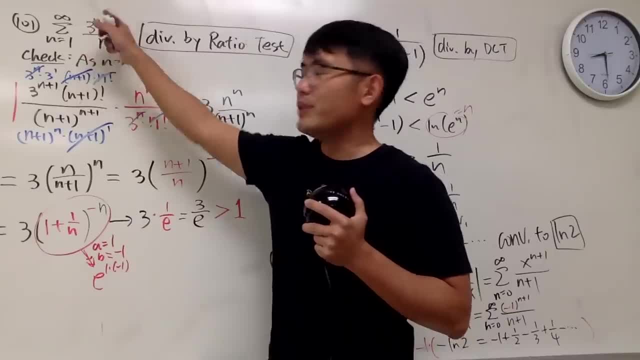 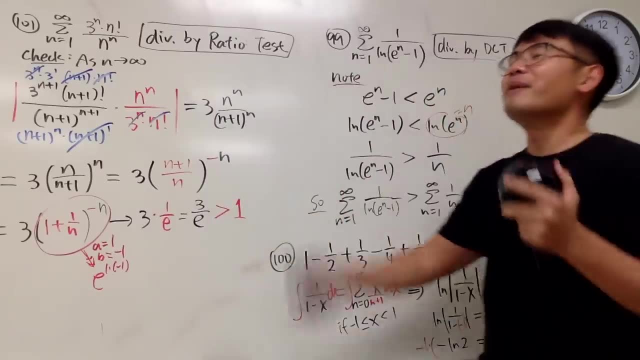 and so on. So this is a 2 to the n and so on, And leave a comment down below let me know what the answer is. Anyway, Oh my God, Oh my God, I'm done. 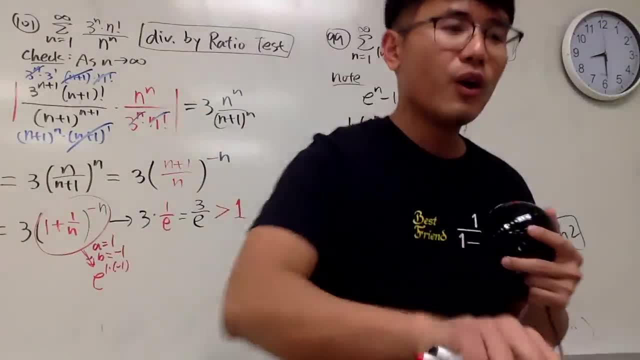 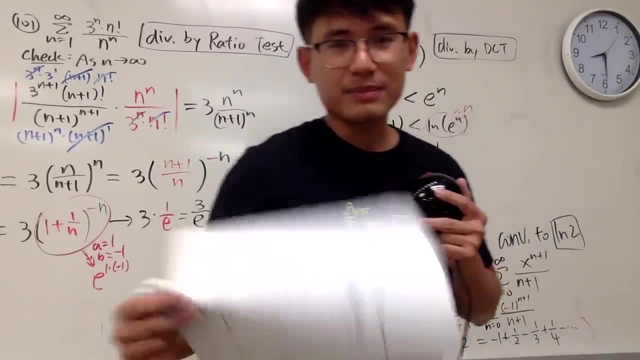 I'm done with all the questions. I'm done with all the questions. Oh my goodness, Oh my goodness. No food, No water, No stop. Okay, I just had to send a text message earlier. 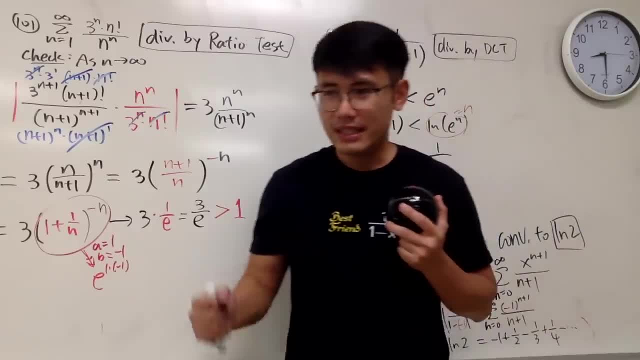 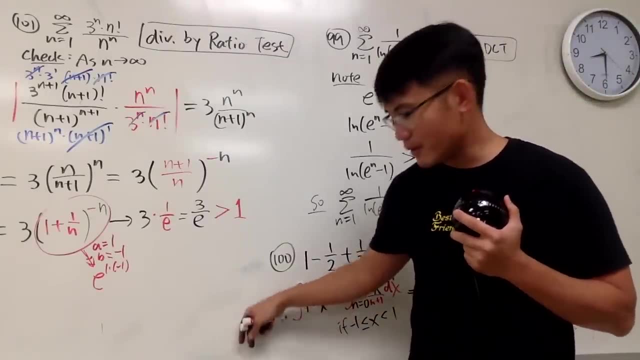 but I, you know, so tired. Alright, so hopefully you guys all find this video to be helpful. Seriously, Seriously. If you have any questions, just leave a comment down below, let me know. And I really wish you guys can subscribe. 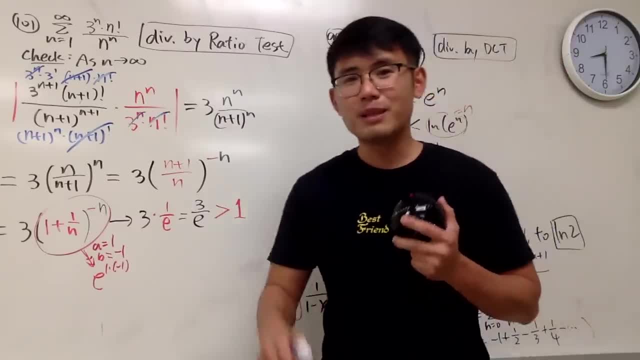 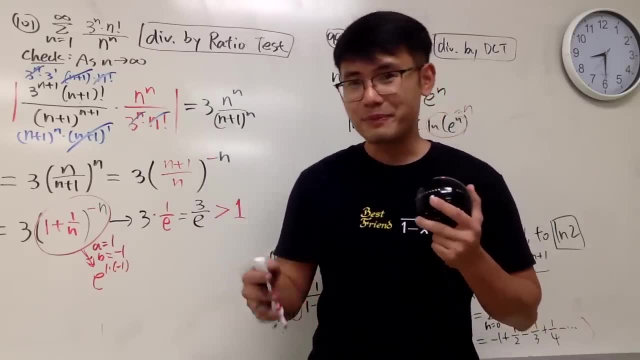 and also help me to share this video so that you know, and you know, I feel like this, this is like worth my time to do all this. I, I feel good. oh, I feel good. 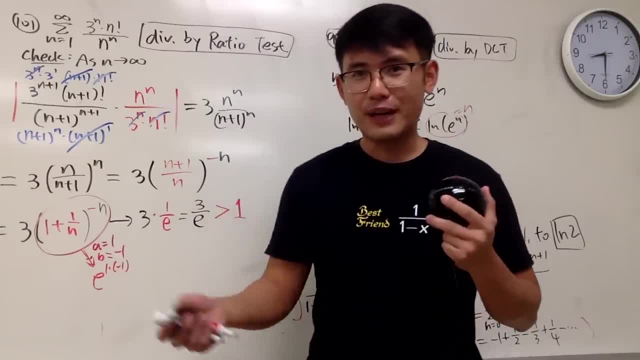 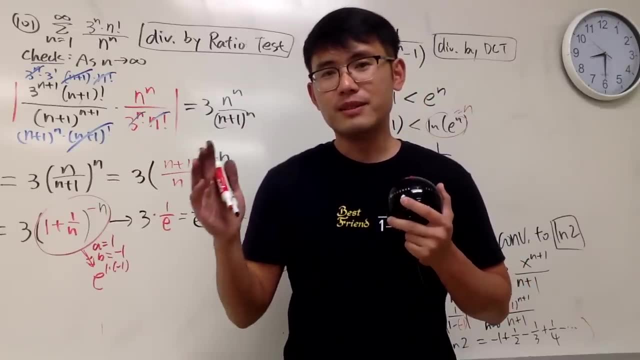 to do all this for you guys. So I feel good to do all this for you guys. I feel happy and then thank you guys. so much for all your support, Thank you for all my supporters, you know. 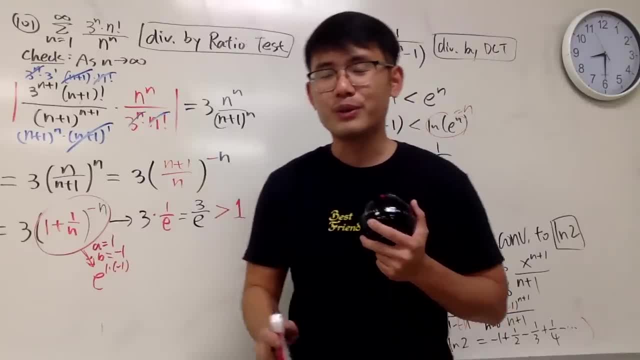 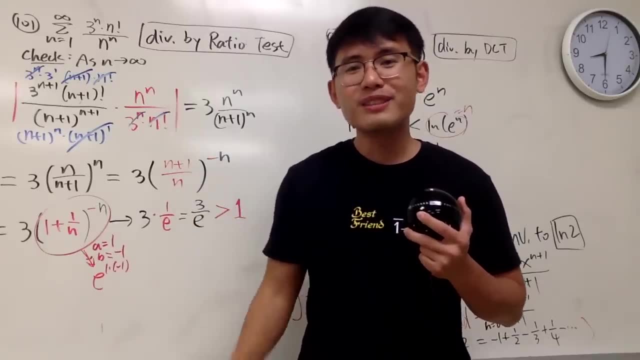 on YouTube, on Twitter, on Patreon. Thank you, thank you, thank you Again, shout out to Lars and Chester, Dr Payan, my girlfriend, and all my subscribers and all my Patreons And, of course, 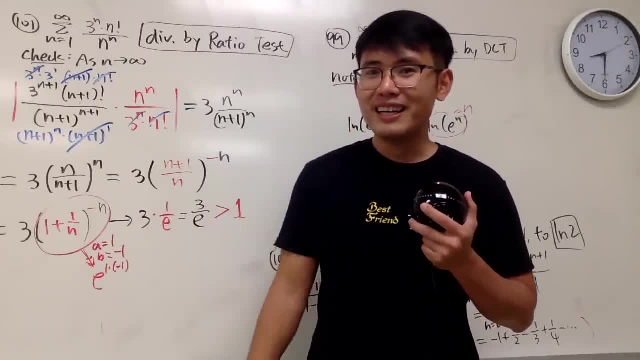 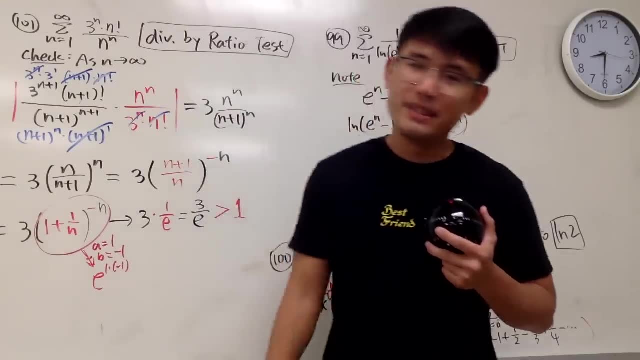 a special shout out to Johnny and Mr Alton from King James School in UK. It's a lot of fun. All right, 8.30.. Six hours and six minutes. oh my god, Whew, I want to have. 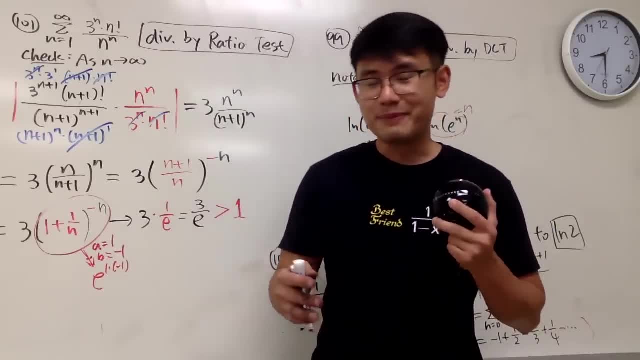 Bye-bye, Bye-bye. I really hope that you enjoy watching. If you do leave a comment down below, Let me know, And I really wish you guys can subscribe and also help me to share this video so that you know. I feel like this is worst, my time to do this. 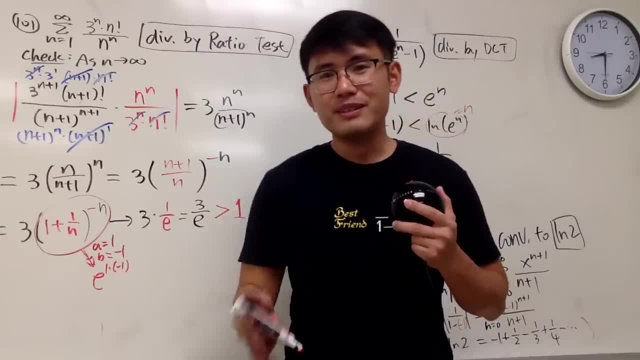 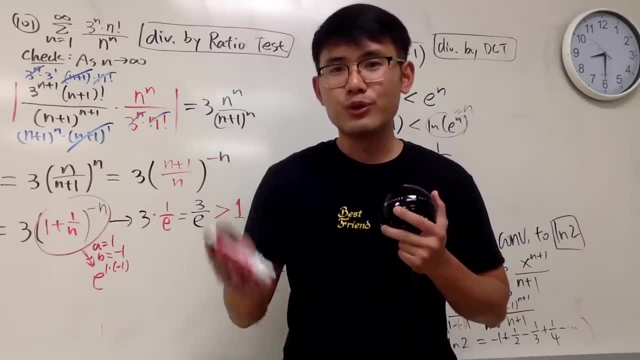 I feel good, though. I feel good to do all this for you guys. I feel happy And then thank you guys so much for all your support. Thank you for all my supporters you know, on YouTube, on Twitter, on Patreon. 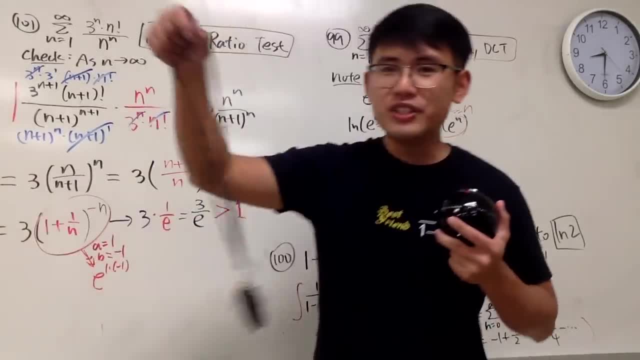 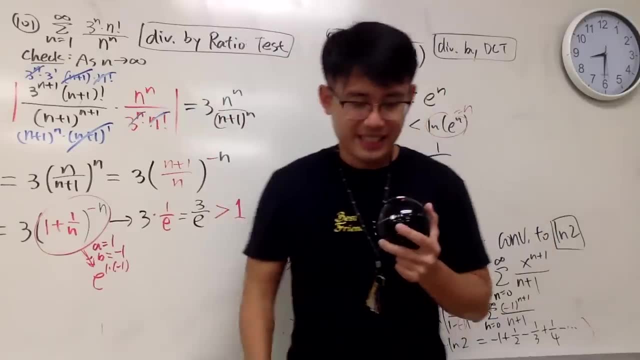 a key chain. I feel like I just want to put something over my head. Whew, Yes, Yes, Yes, Yes, Yes, Done, All right, so done, Yes. So hopefully you guys don't ask me for like.